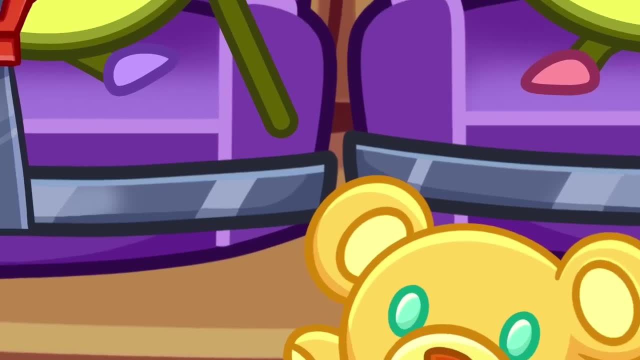 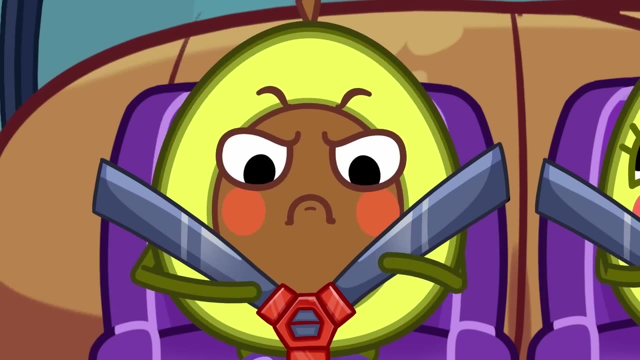 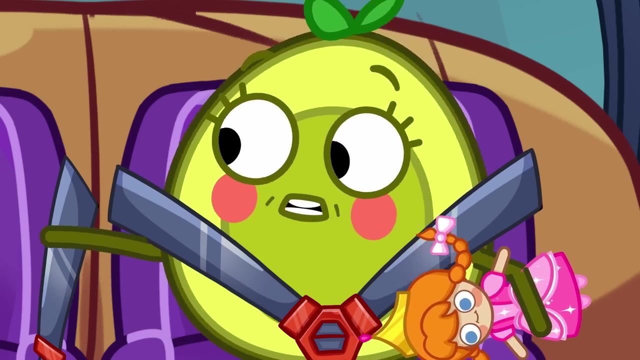 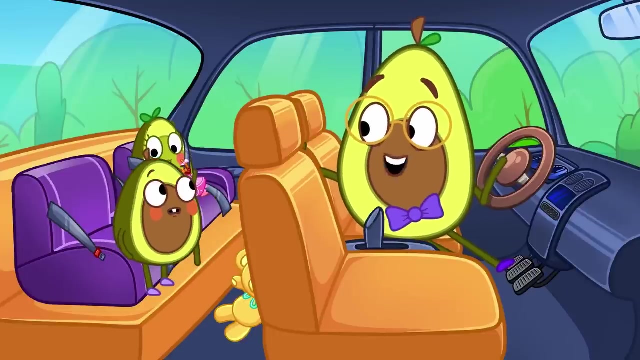 Pit dropped his teddy bear And now he can't reach it. No, Pit, Don't leave your seat, Dad. Dad, Pit hasn't fastened his seatbelt. Pit, fasten your seatbelt, please. Seatbelts, keep you safe. 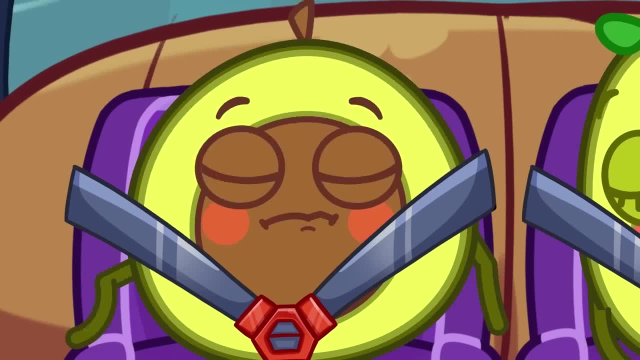 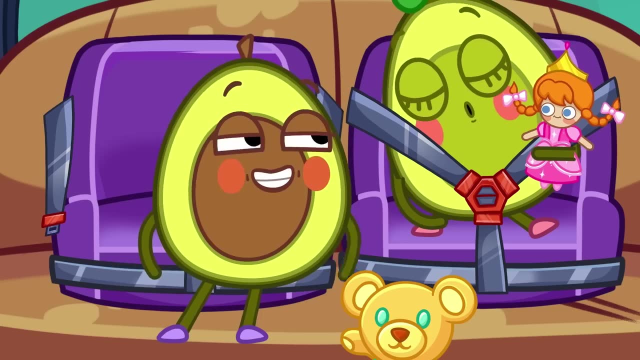 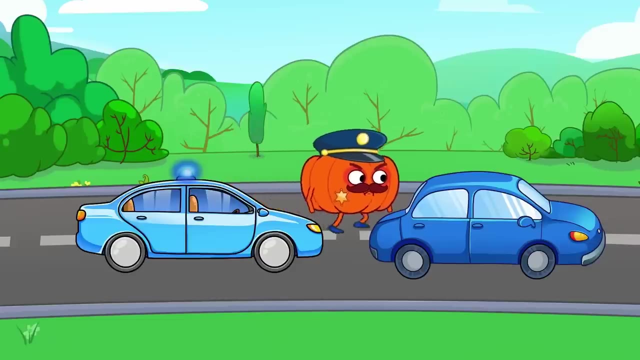 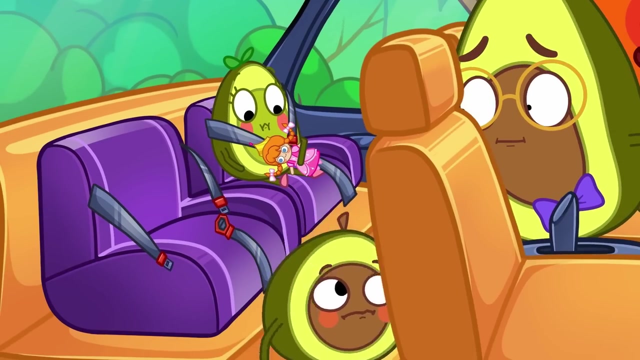 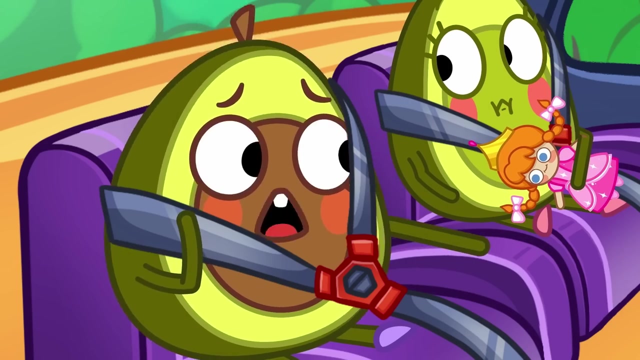 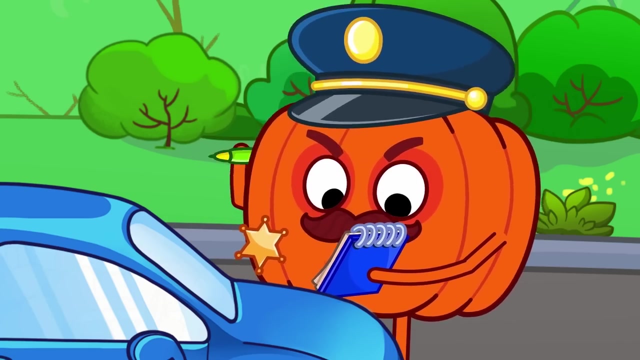 Pit. that isn't a good idea. Officer Pumpkin isn't very happy. What is it? Pit wasn't wearing a seatbelt. Pit, are you hurt? I'm not, but my bear is Daddy has to pay a fine because of Pit. 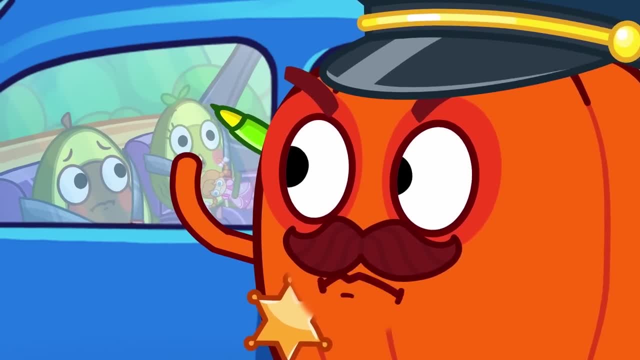 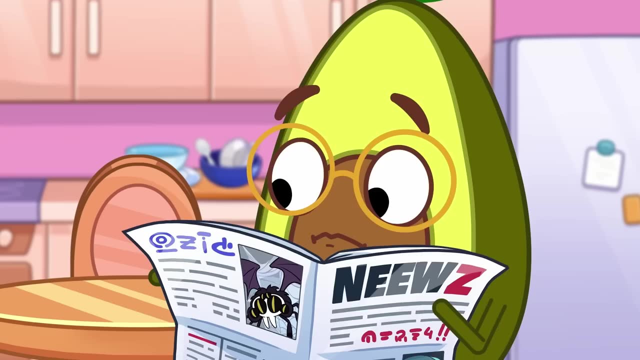 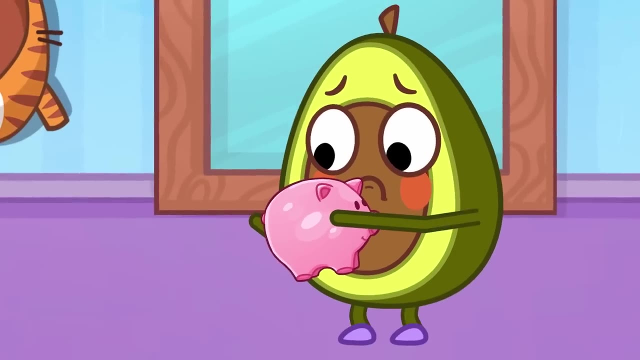 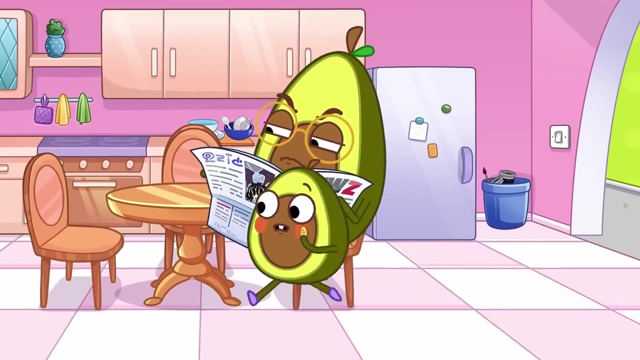 Never unbuckle your seatbelt. It's dangerous. What's wrong with Daddy? Oh, the fine. That's why Dad is still angry. Pit wants to help Daddy pay. The offender must pay a fine. Okay, Pit, Let me explain this to you. 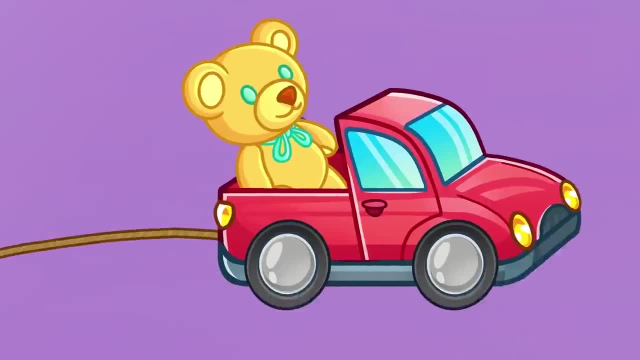 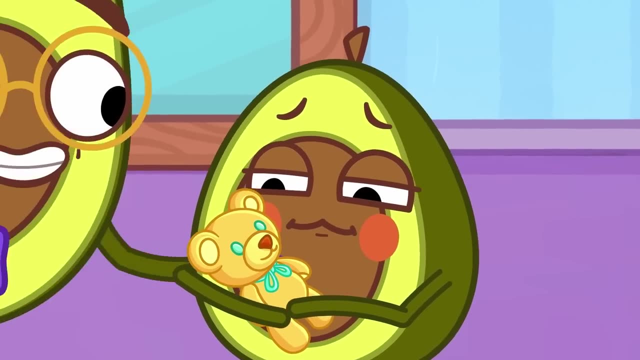 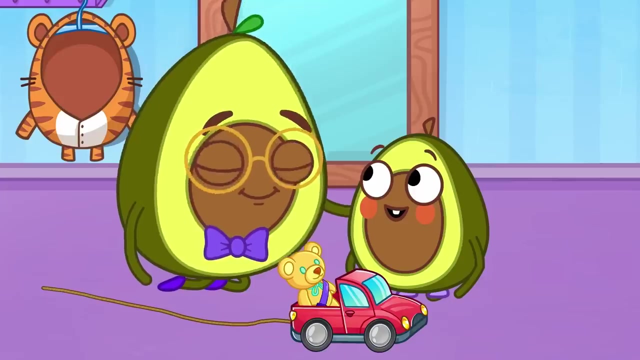 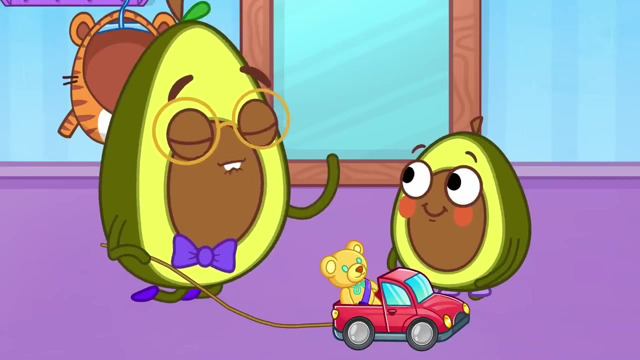 Let's start our crash test. Here's what happens: without a seatbelt, The passenger isn't protected. I'm worried about you, Not about the money. Remember: the seatbelt is for your safety. Everyone's wearing a seatbelt now. 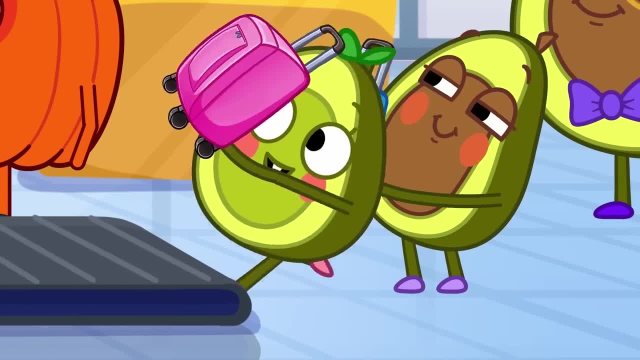 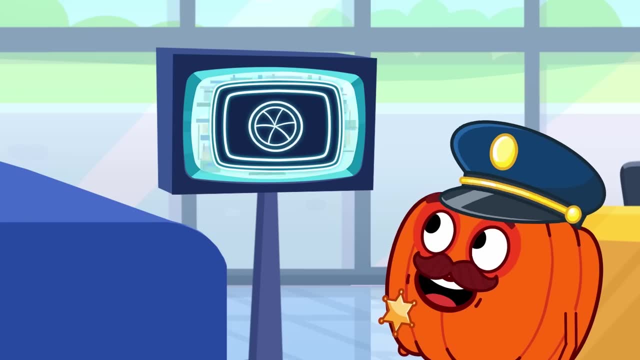 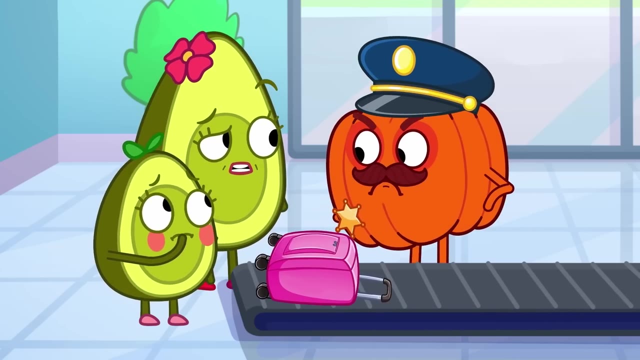 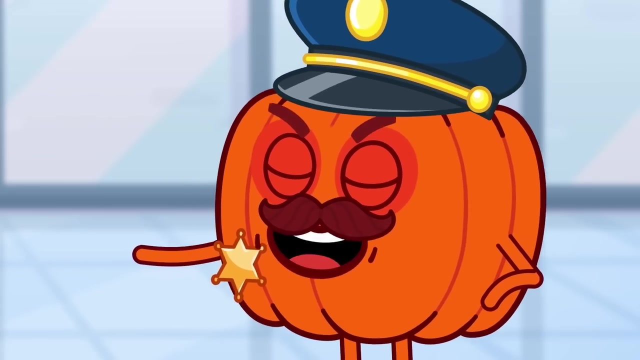 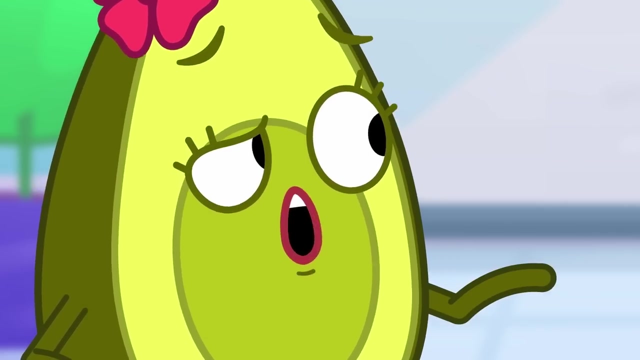 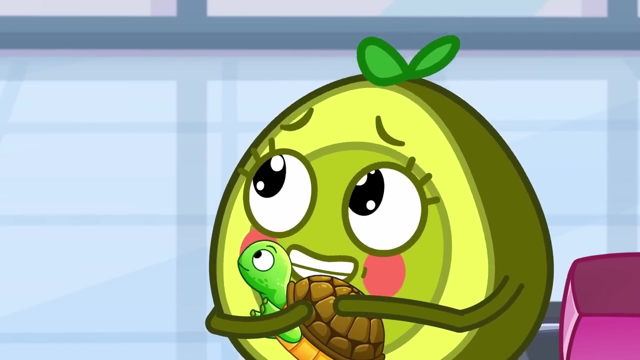 The avocados are at the airport. There's something in Penny's suitcase. It's her pet turtle. It's forbidden, Please, Officer. what can be done? You can leave your pet at the pet hotel. Your pet will be much happier here. 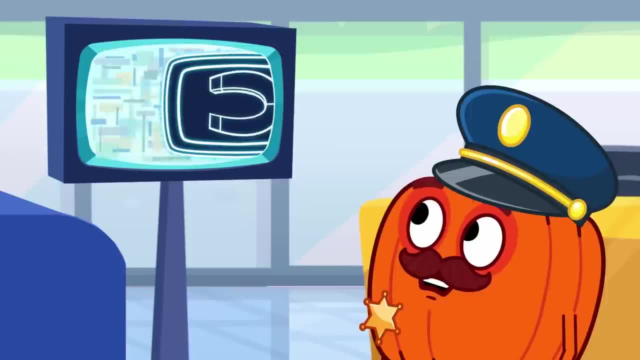 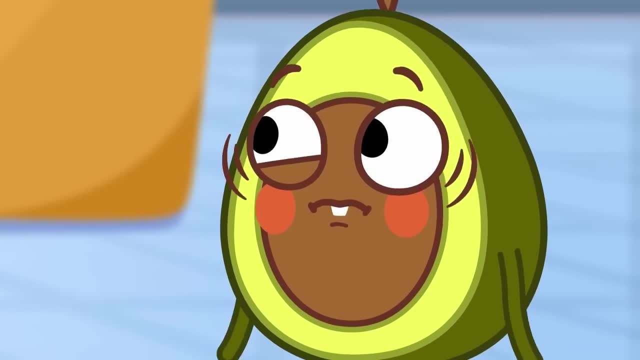 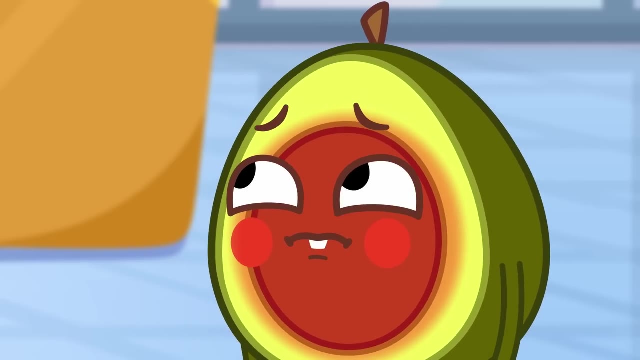 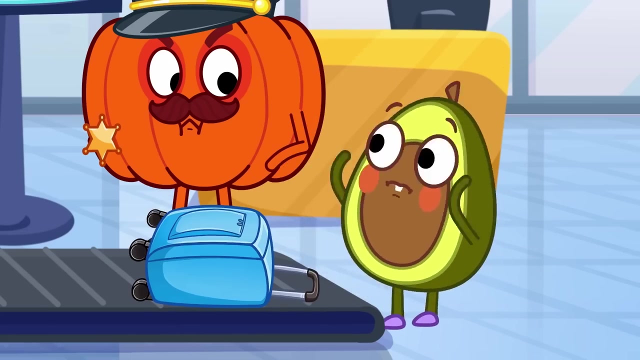 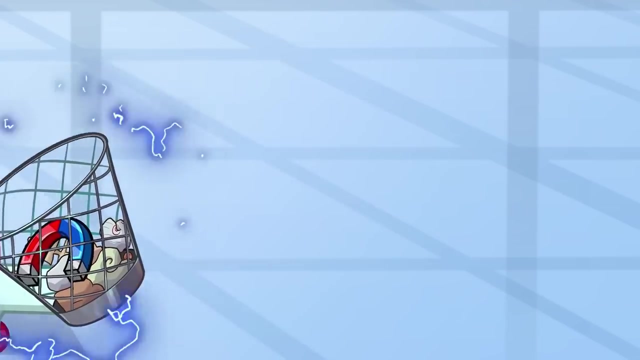 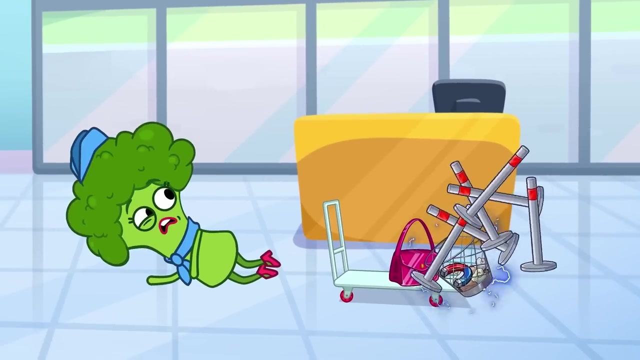 That's not true. There's something in Pit's suitcase. You can't bring that on the plane. Pit Magnets aren't prohibited. That's much better. Oh, What's in Daddy's suitcase? Fireworks, Oh Daddy. 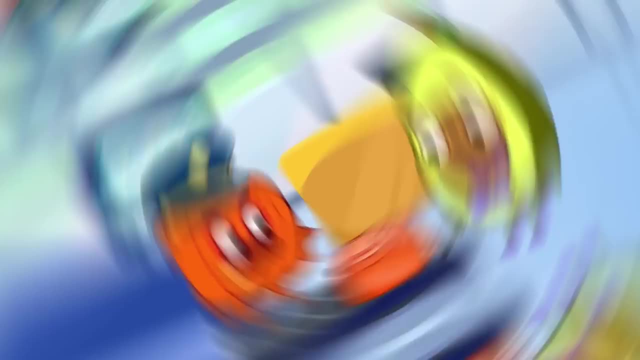 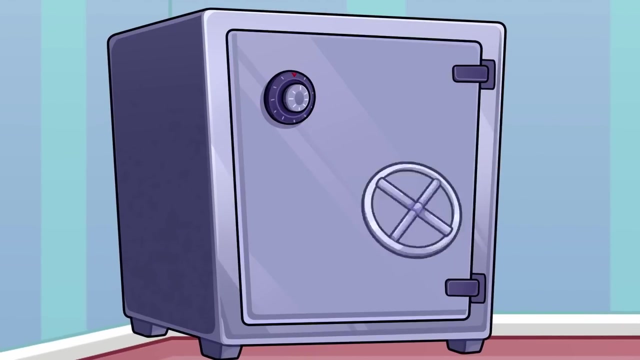 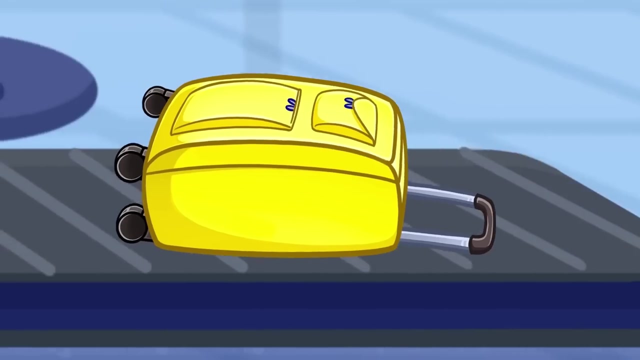 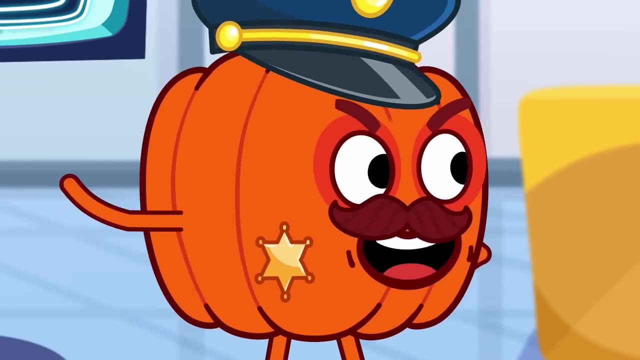 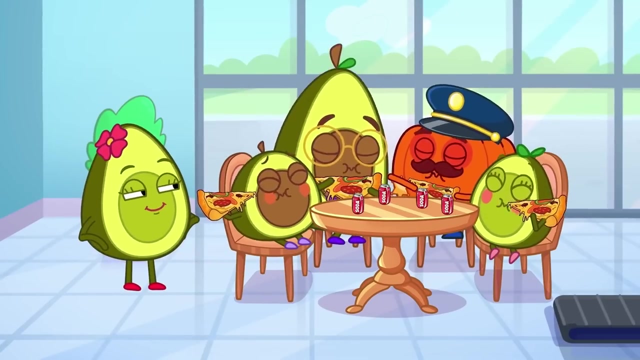 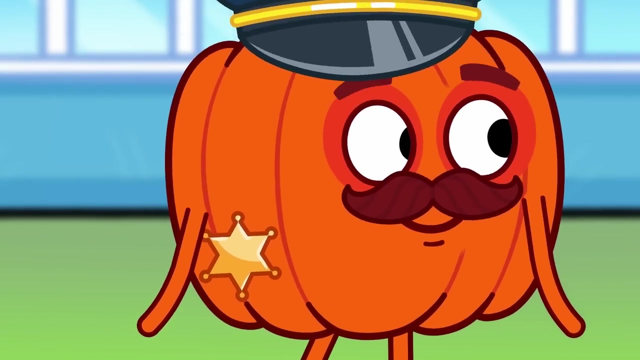 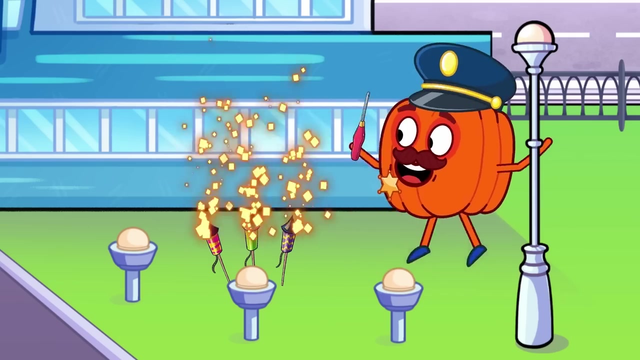 Fireworks are not allowed on the plane. Sorry, Let's put them somewhere safe. Watch and learn What's in Mommy's suitcase. It's forbidden. You can eat that now. Have fun. Come on, Officer Pumpkin. It's raining, Penny. 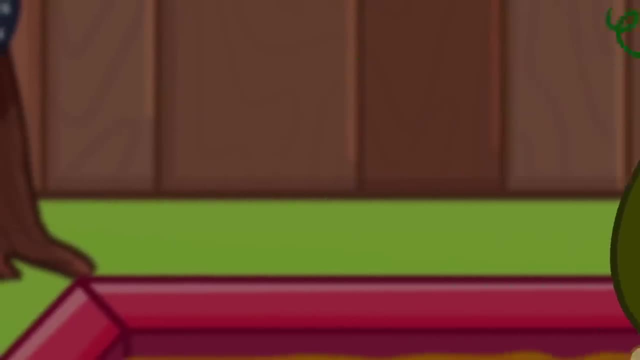 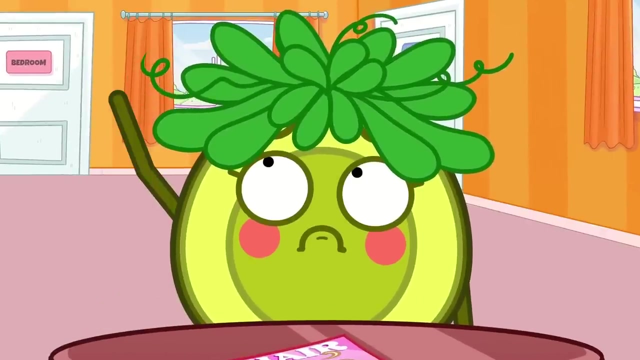 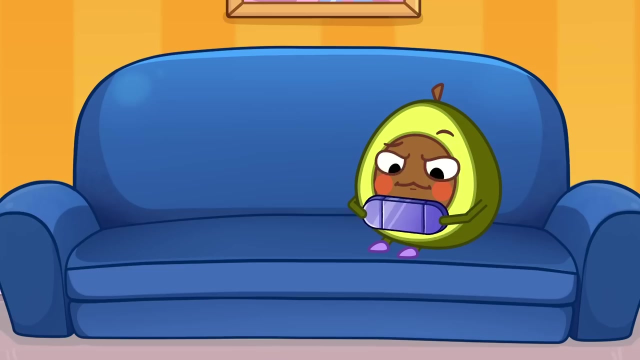 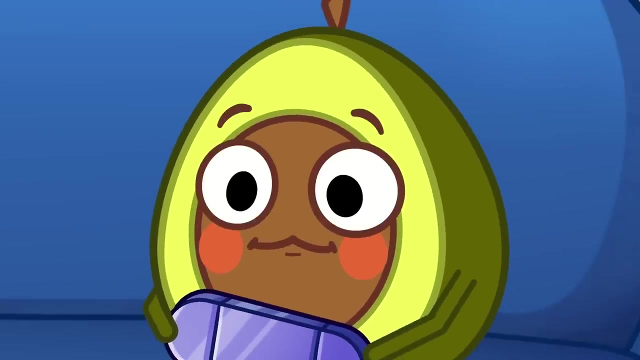 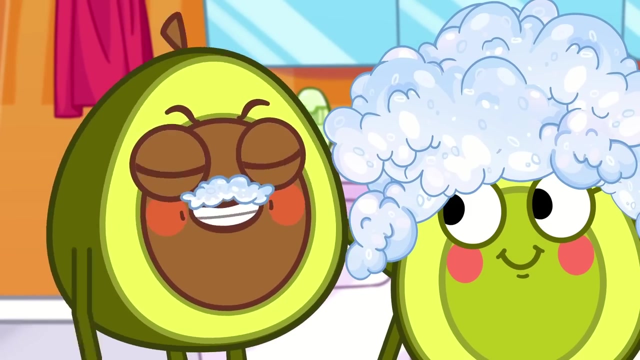 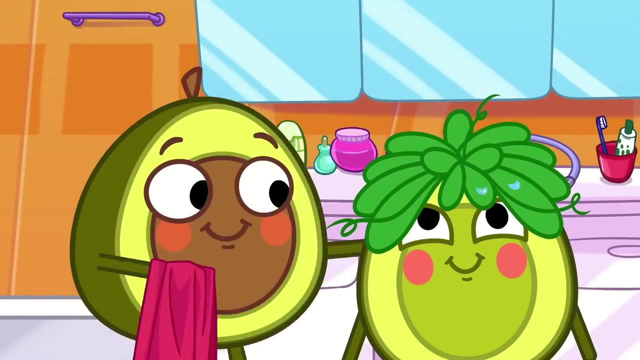 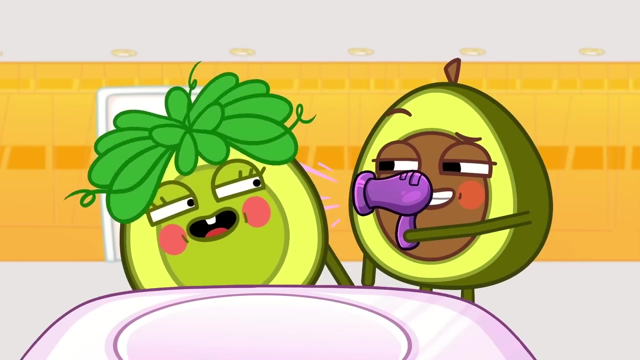 Time to head inside. Look at all the hair Hair Pit. will you help style Penny's hair? First you need to wash the hair, Then you rinse out the shampoo And finally you dry it. Now for the fun bit. 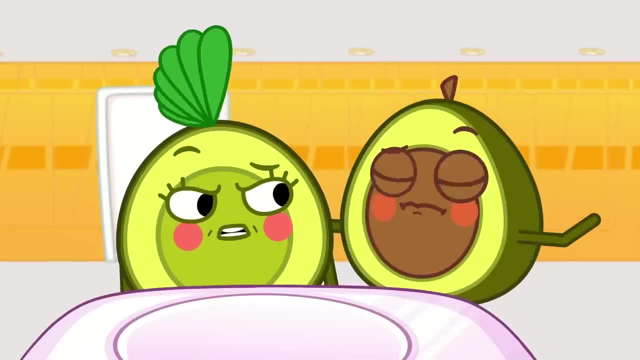 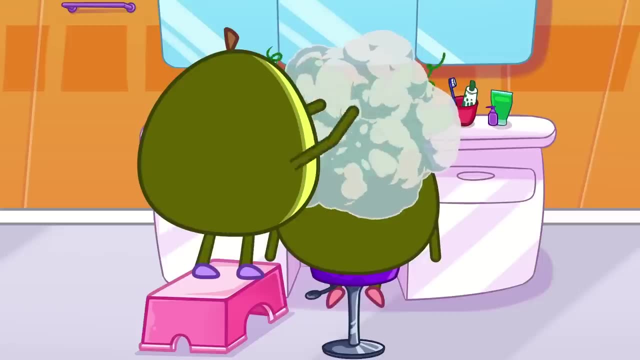 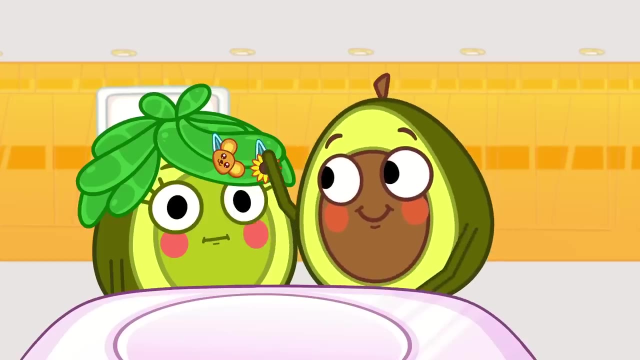 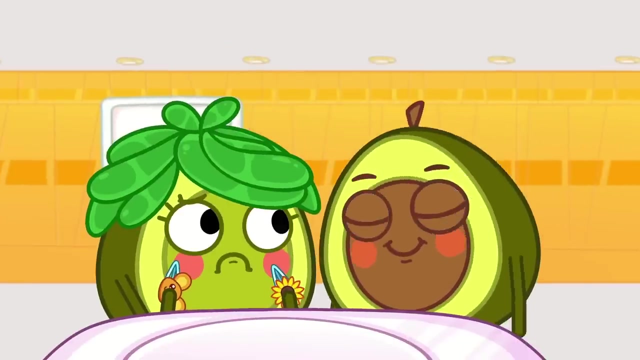 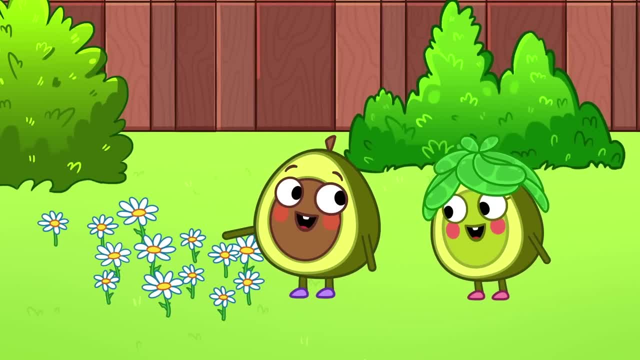 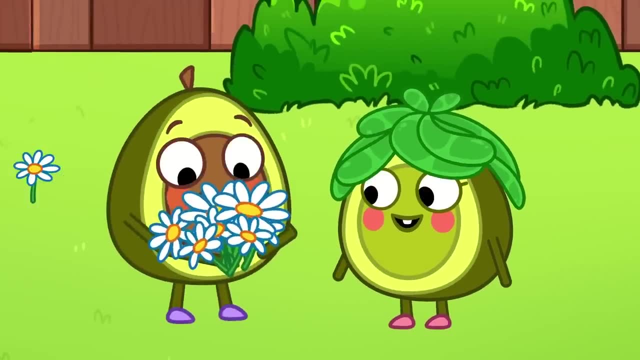 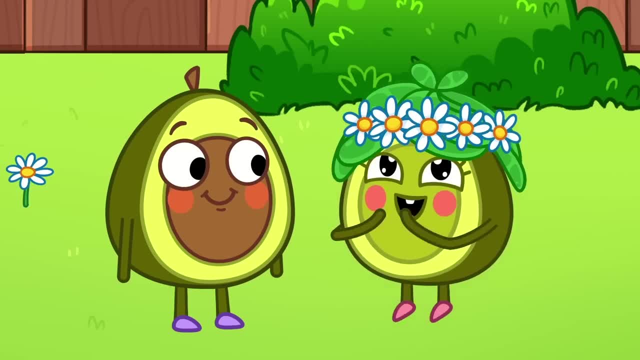 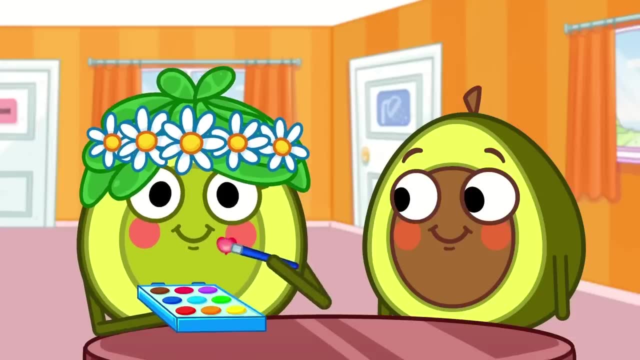 Bye Penny. Bye Penny, See you later, Pit. Bye Time, Reacher. Bye My Love. See you later, Penny. Wow, You're graphic Due. Yes, And look at this, You're Gosh a Uglystone. 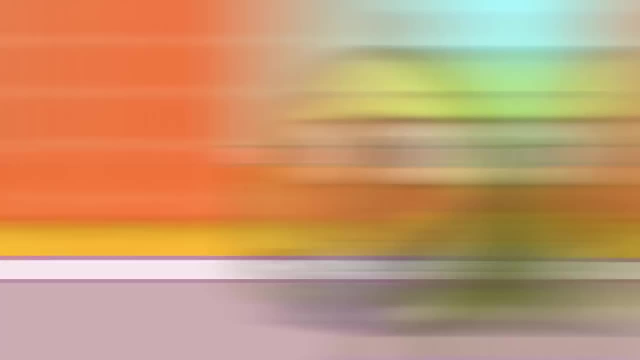 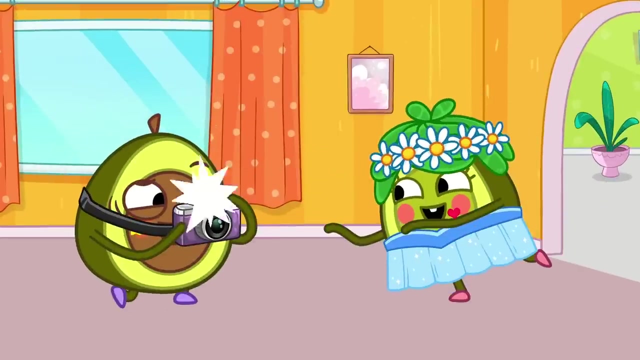 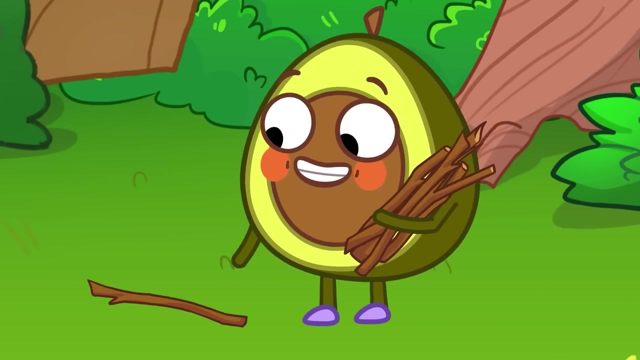 You look like aNaughty correr Yellow. Yeah, Uh, huh, I mean this And this. Ooh, Penny's ready for some pictures Looking great. Penny Pit's collecting wood for a picnic Pit. sees a spider. 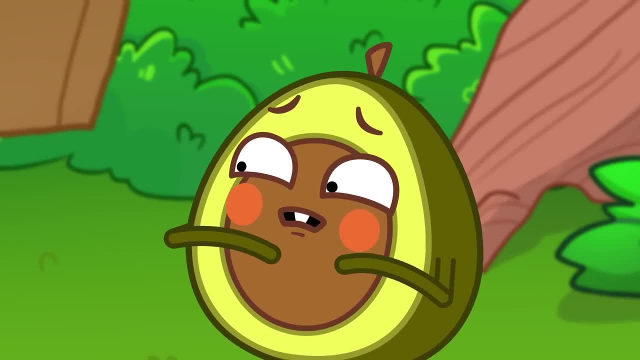 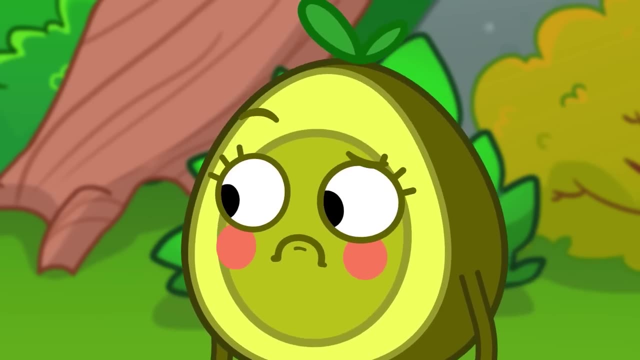 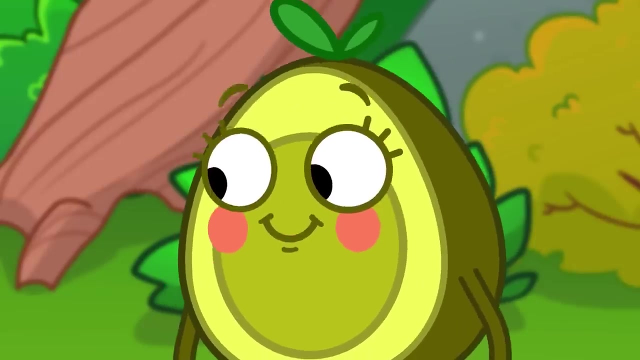 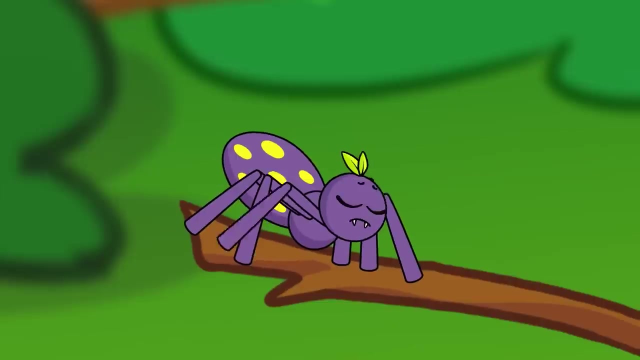 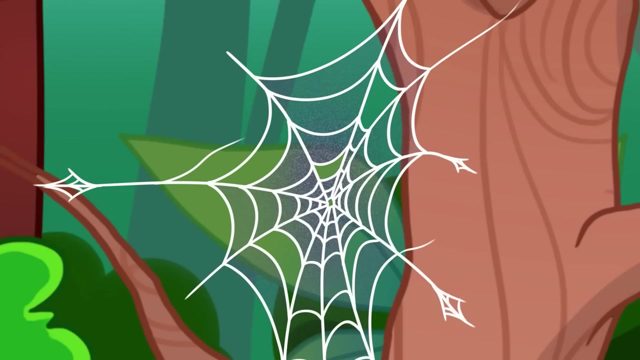 Woo, There's a monster. Help, Penny Pit's afraid of the spider. Oh, where Penny's not afraid, The spider wants to go back to its web. This is where the spider lives. Spiders don't live in a web. 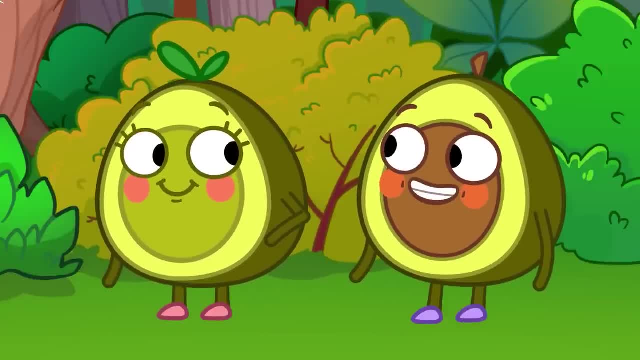 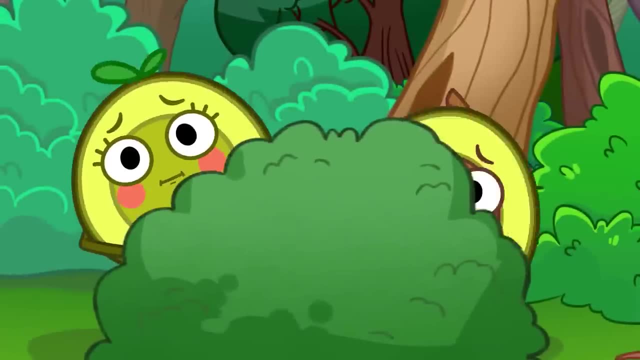 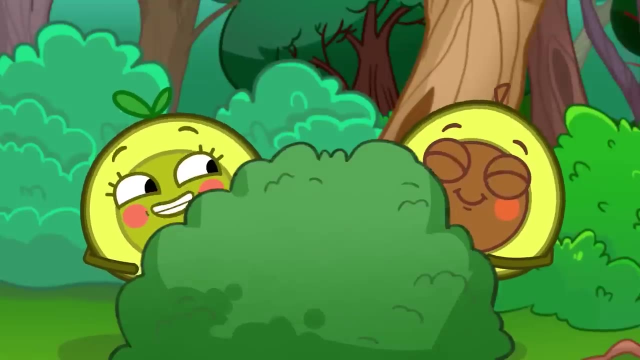 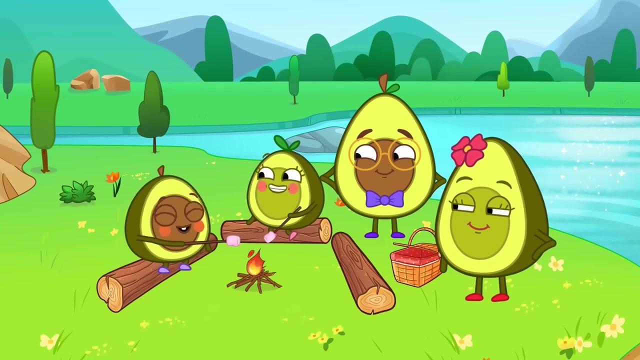 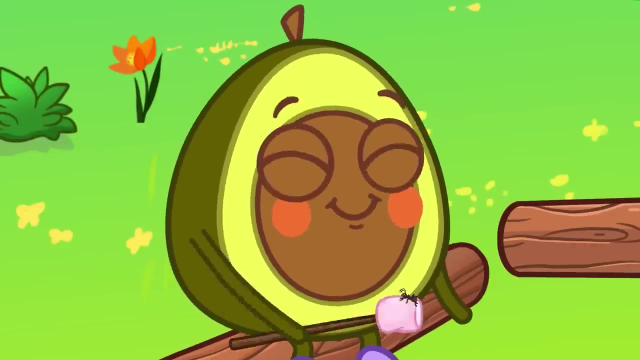 They don't attack unless disrupt. Oh no, Mosquitoes. Where do they go? They're caught in the spider web. Spiders hunt mosquitoes. They're useful. It's time to roast marshmallows Twice a day. eat handfuls instead of willy-nilly. 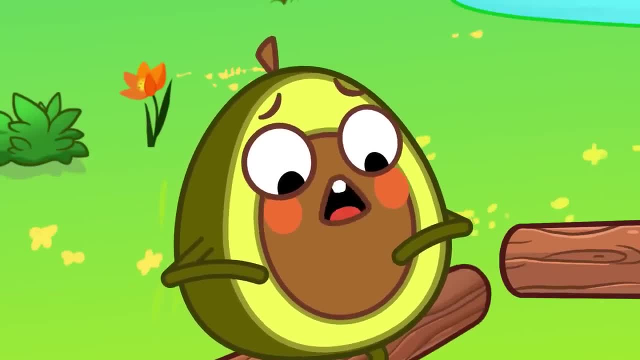 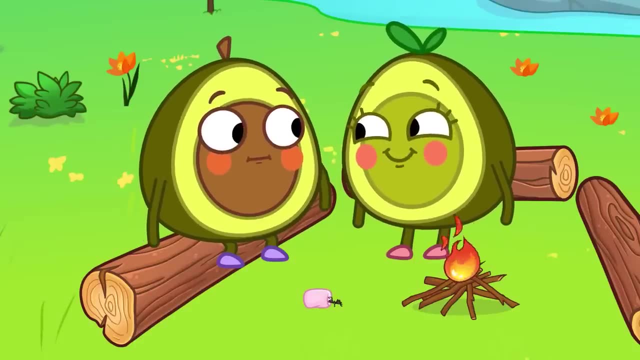 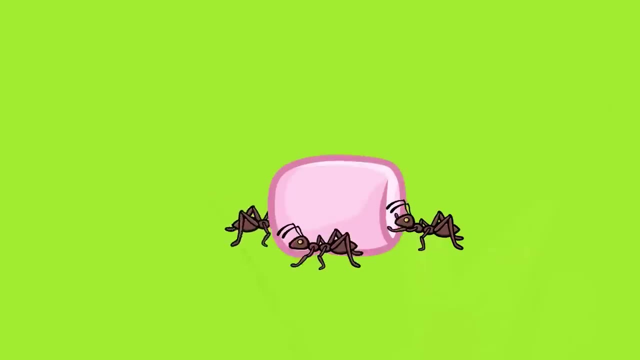 All right, I'll just rob you of them. It's time to eat marshmallows. What's on Pit's marshmallow? Oh no, That monster has my marshmallow. It's an ant. They're not scary, They are also very strong. 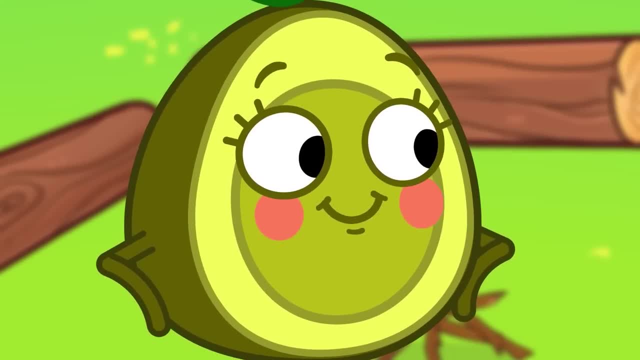 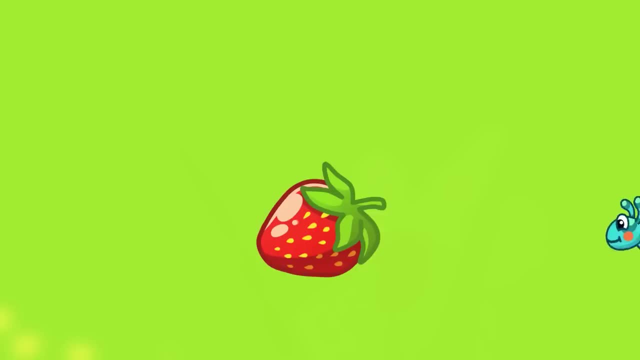 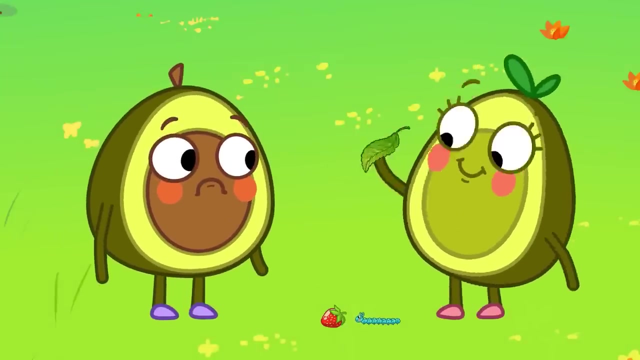 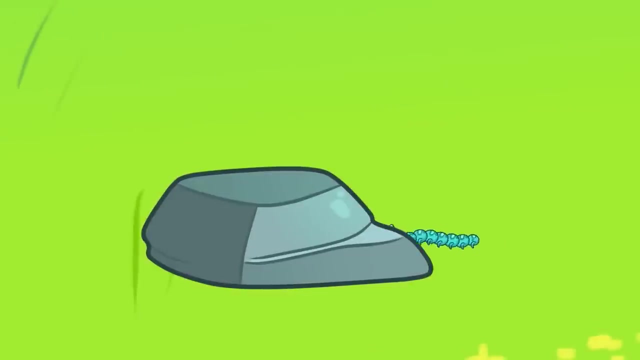 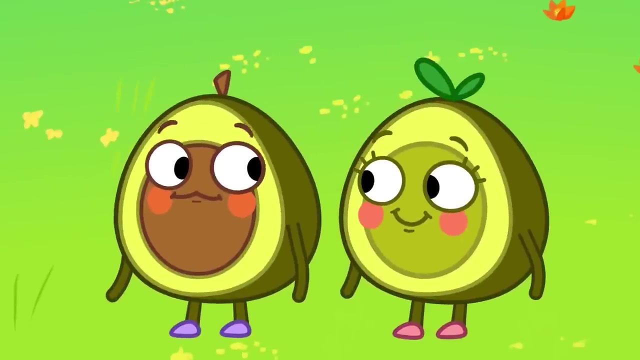 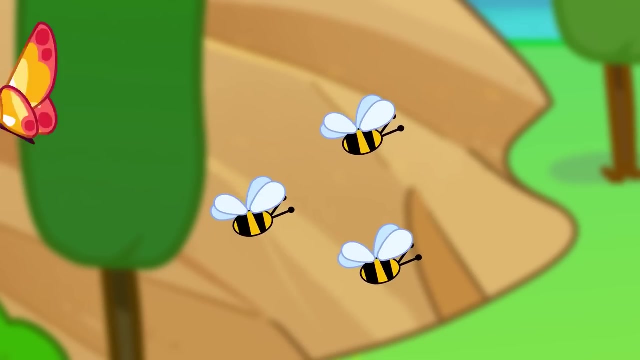 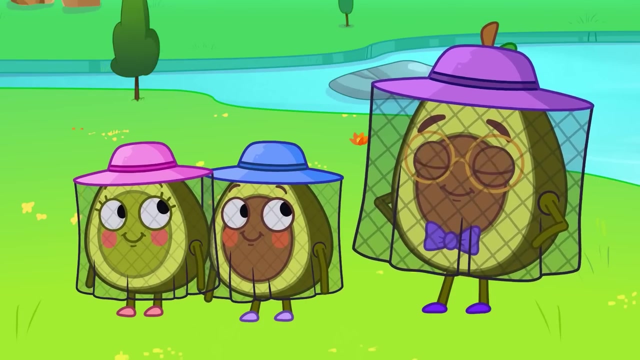 And always work together. That's a caterpillar Run. It won't bite anyone, It only eats leaves. Look it changed: Caterpillar is turning to butterfly. Those are bees. Don't be scared Pit. It's better not to approach bees without protection. That's because bees can sting. 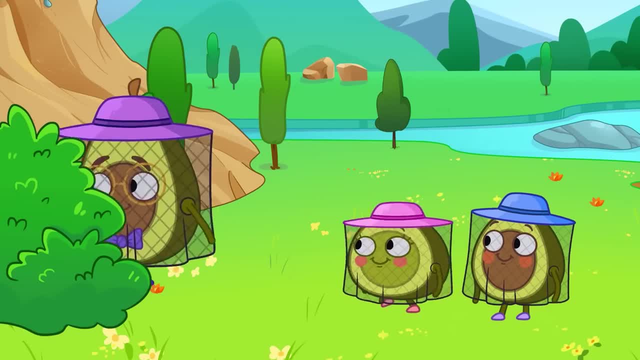 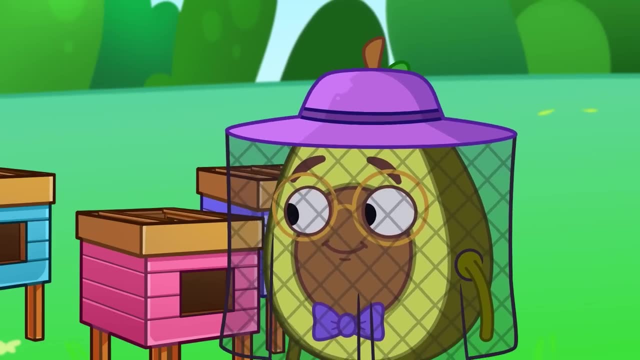 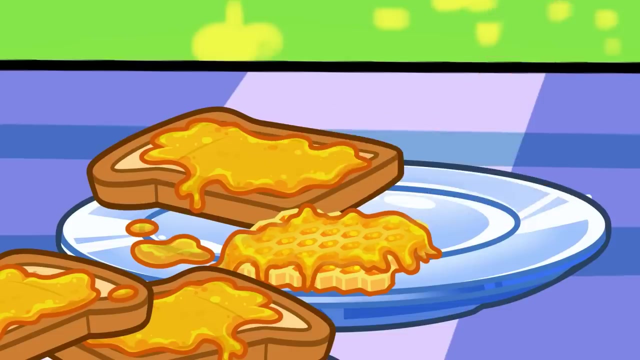 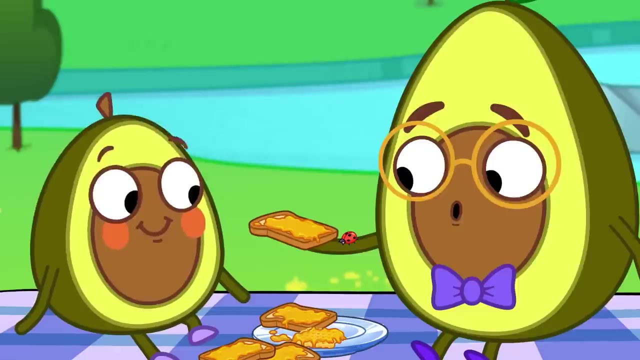 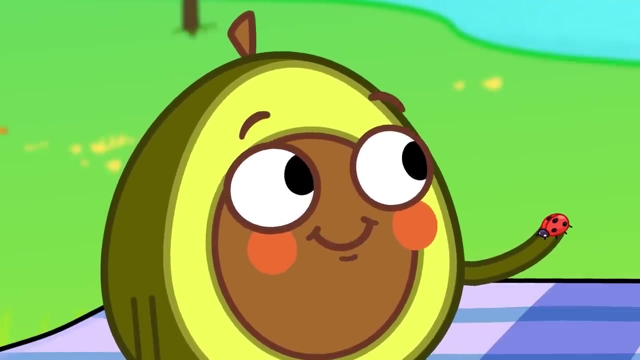 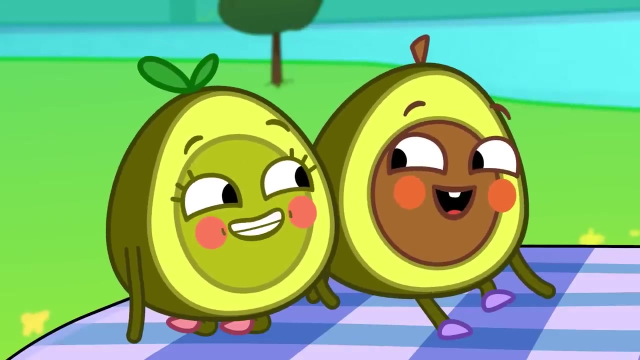 Bees are useful. They make delicious honey. They make their honey in hives. There's another insect. Is it a bee Pit? No, it's just a ladybug. It's a bee Pit. It's not scary. It's fun learning about nature. Pit and Penny are making a car out of blocks. 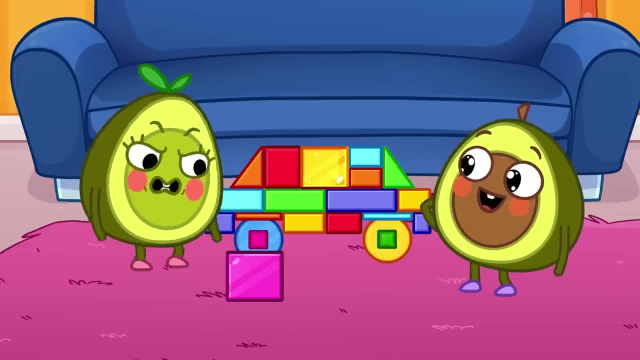 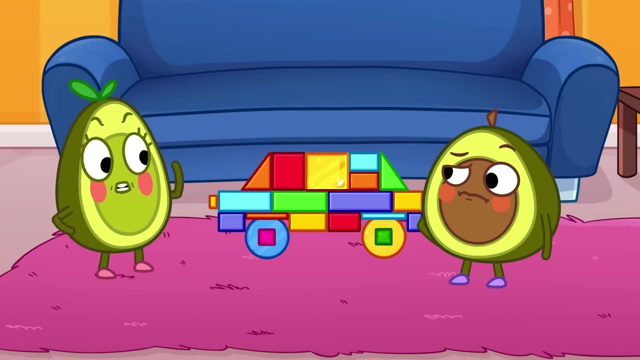 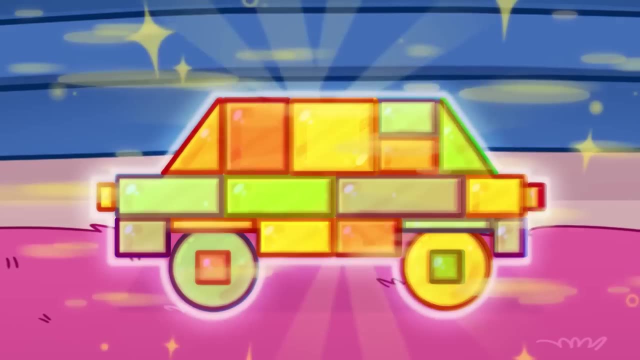 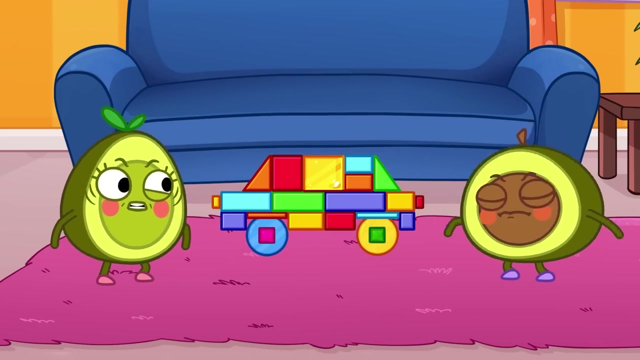 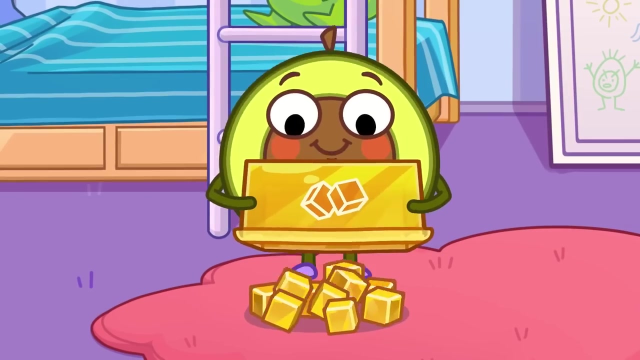 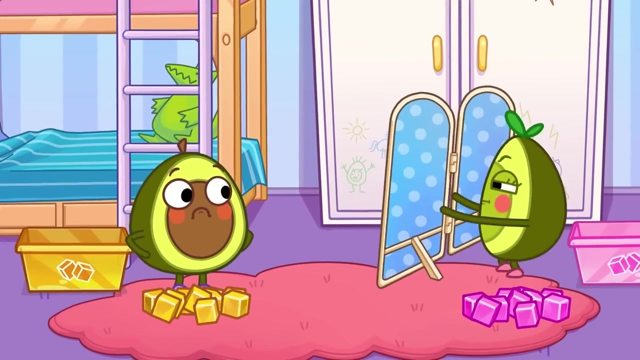 Pit adds a gold block, But Penny wants a pink block. Penny thinks a pink car is better, Pit wants a gold one. Let's have a competition to see whose car wins. Pit will make a gold car, Penny will make a pink car, Penny will make a pink car. 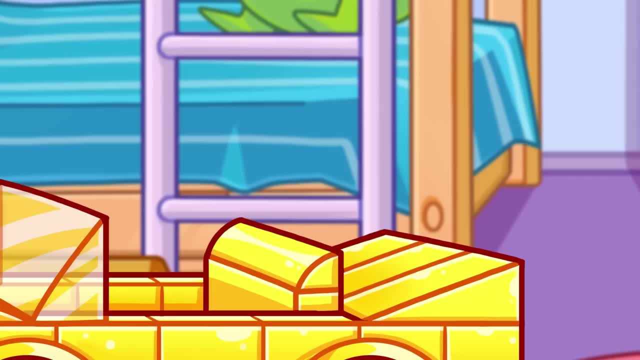 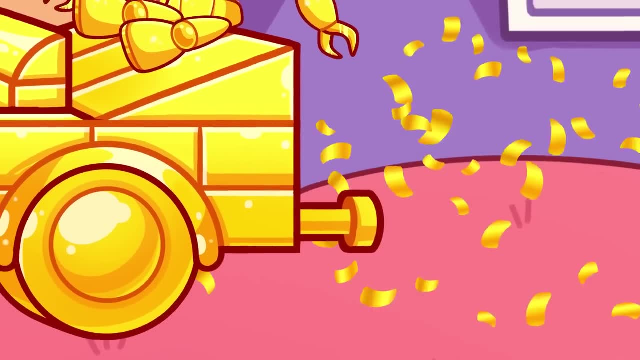 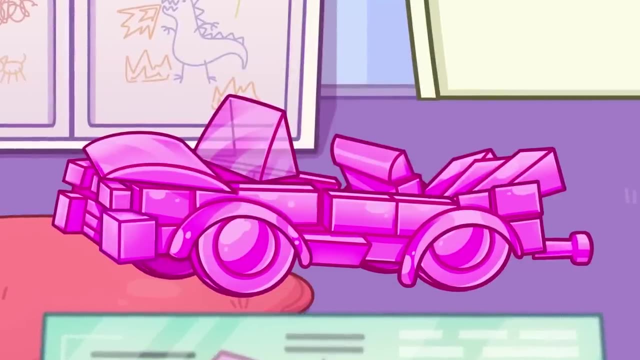 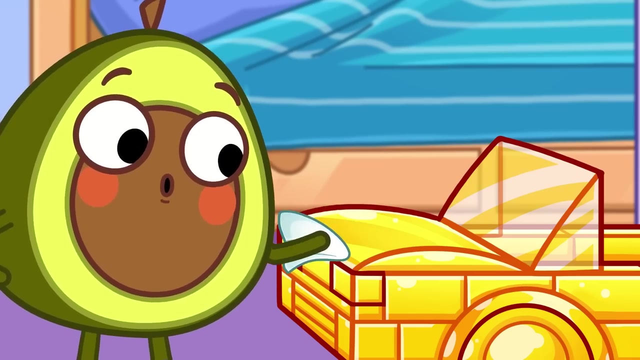 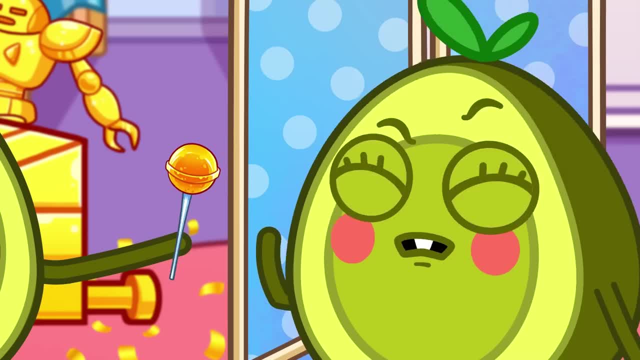 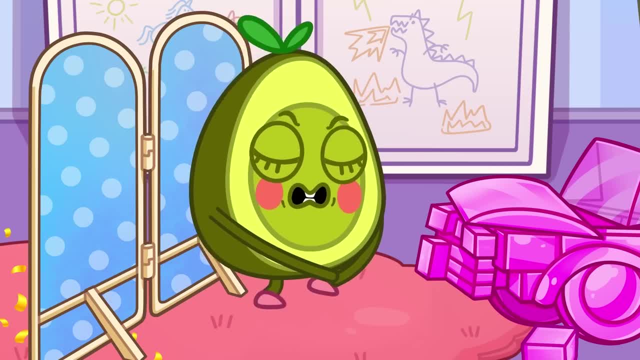 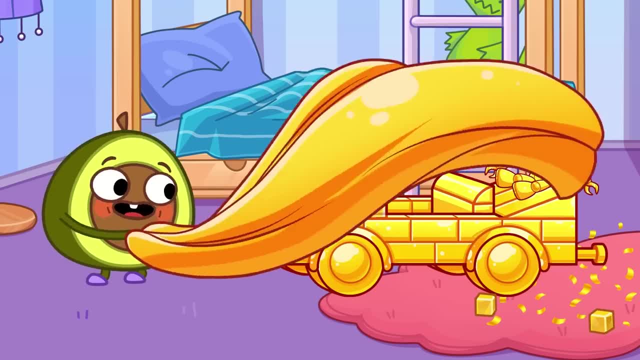 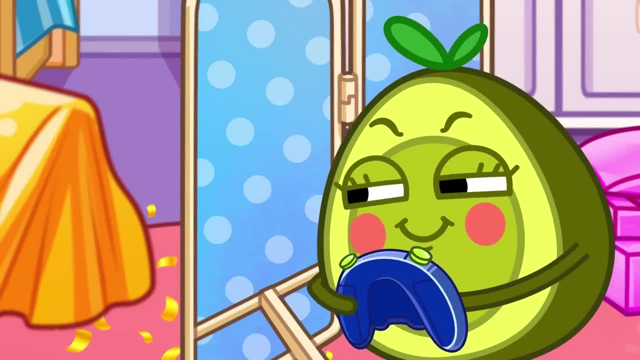 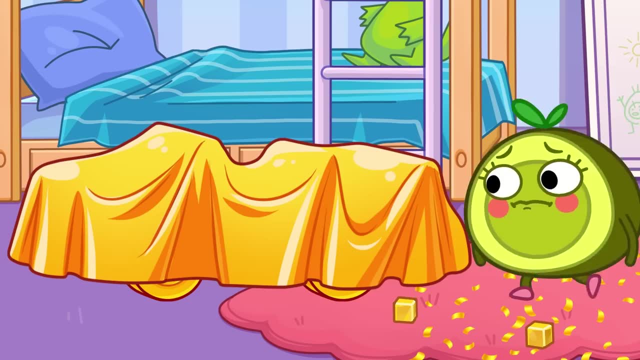 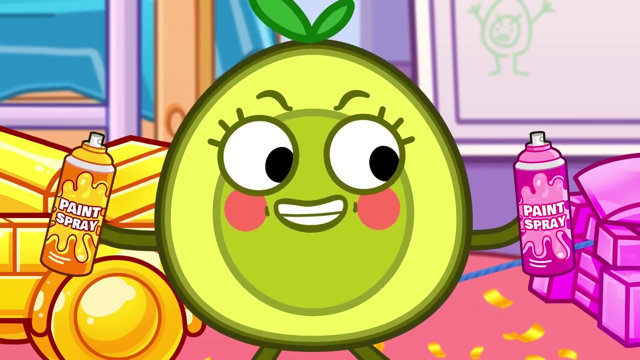 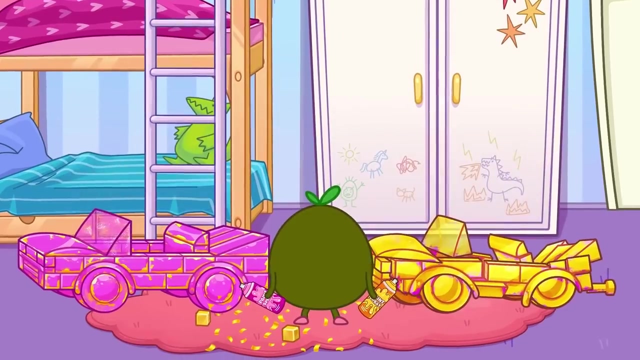 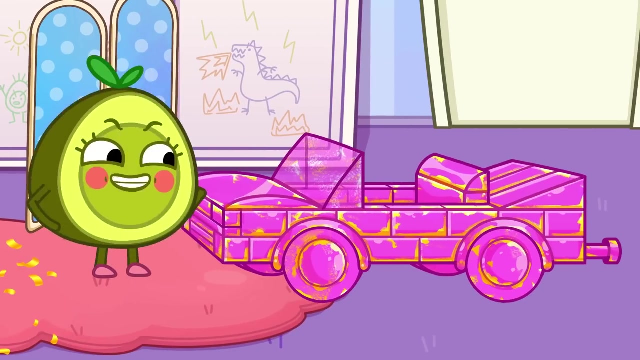 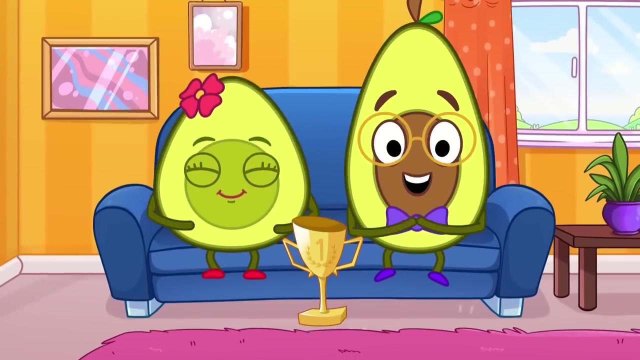 Your car needs to look more like Pit's. Your car needs to look more like Pit's cupcake. Then she'll change the cars with spray paint. Pit's car is pink, Penny's car is gold. Oh, Penny, that's cheating Time for the competition. 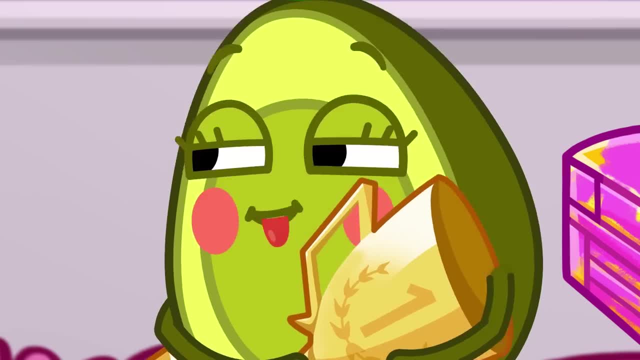 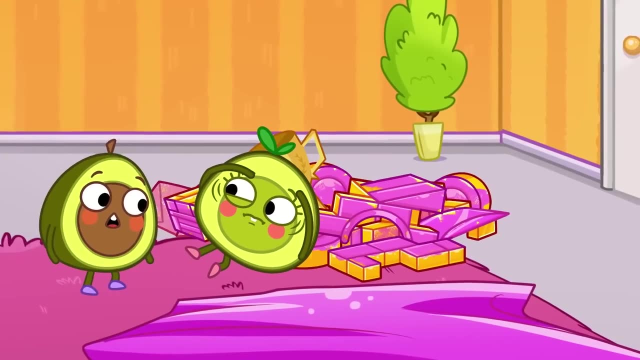 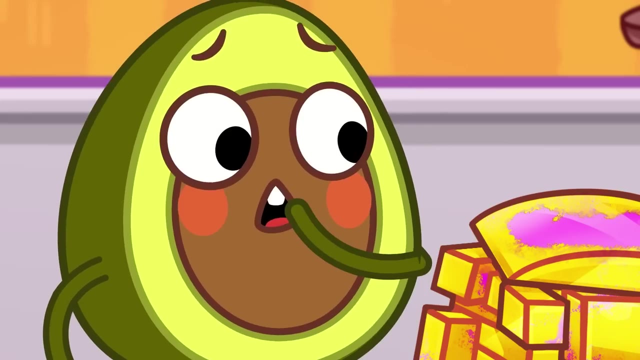 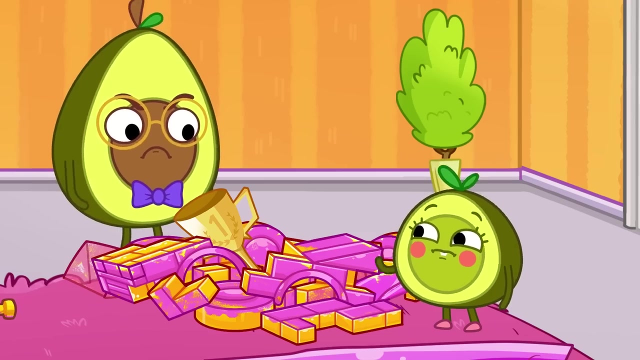 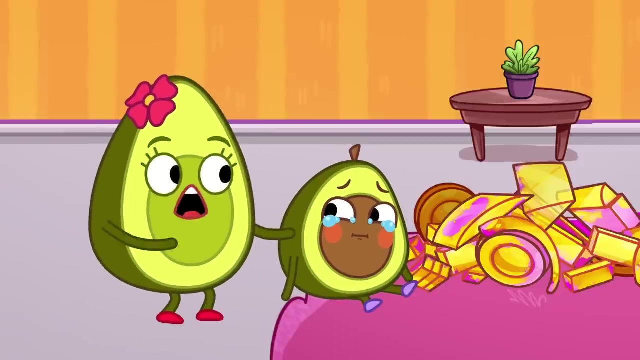 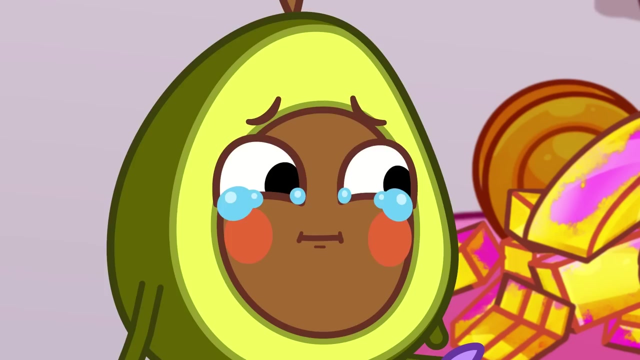 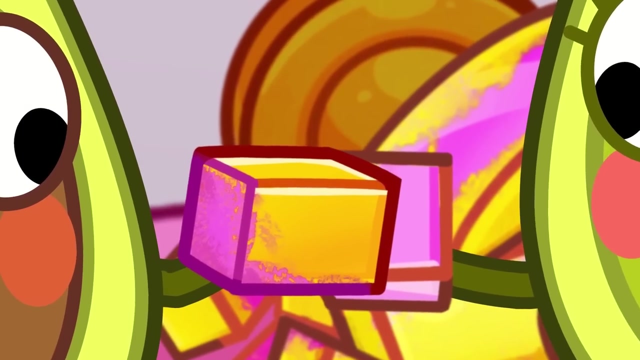 Pit knows Penny cheated. Now we can see the gold blocks And Penny's pink ones. Penny, that wasn't fair. Pit worked very hard to make this car. Penny, what can you do to make it better? Let's see what Pit and Penny did. They made a gold and pink car. 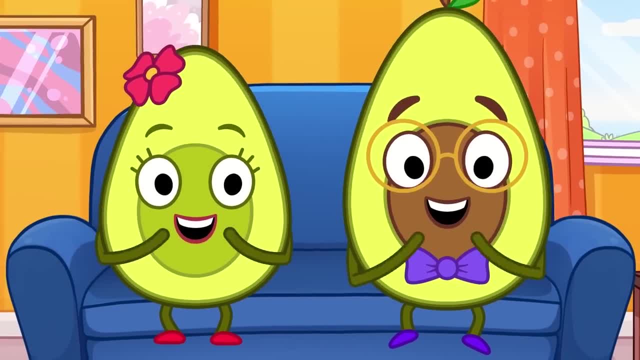 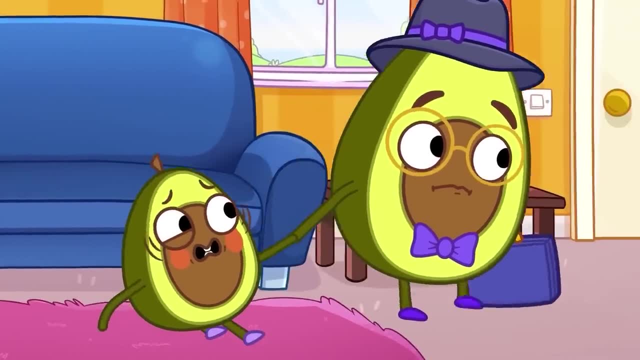 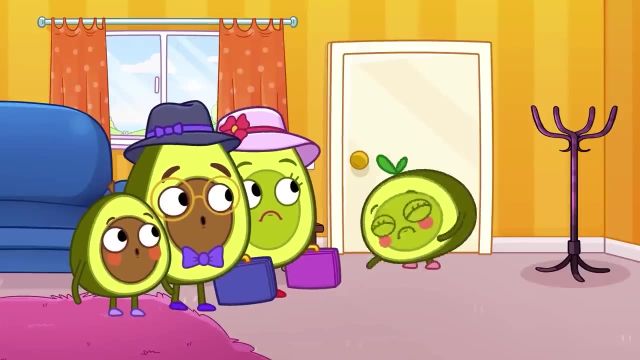 Working together makes them both winners. Penny is upset. Pit is upset too. Mommy and Daddy are going away. Please don't leave us. Who will take care of Pit and Penny? This is Mrs Apple. She's your babysitter. 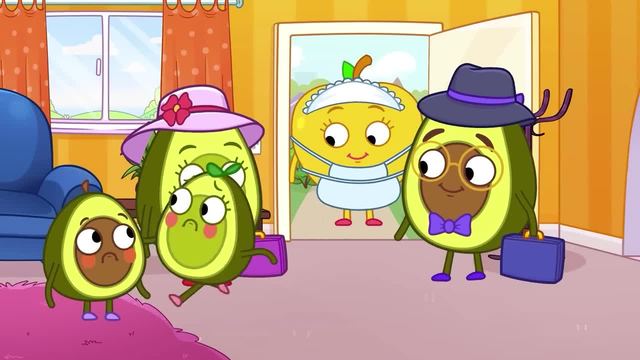 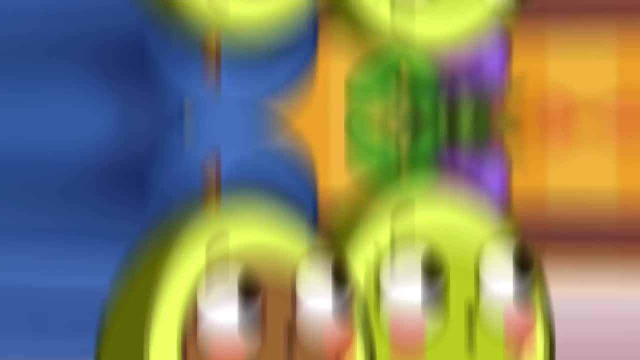 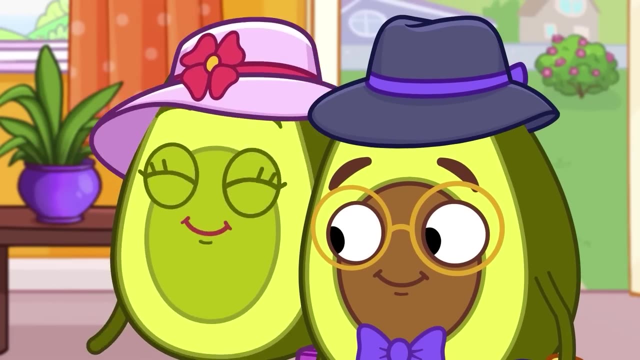 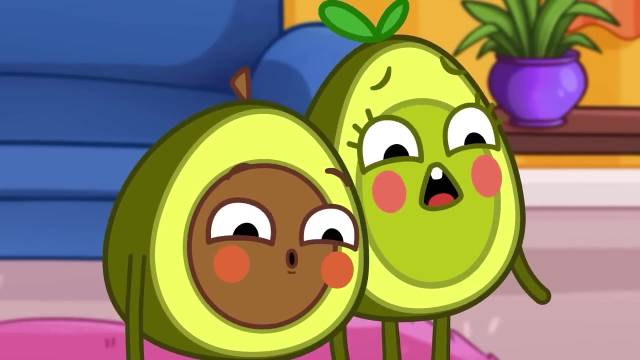 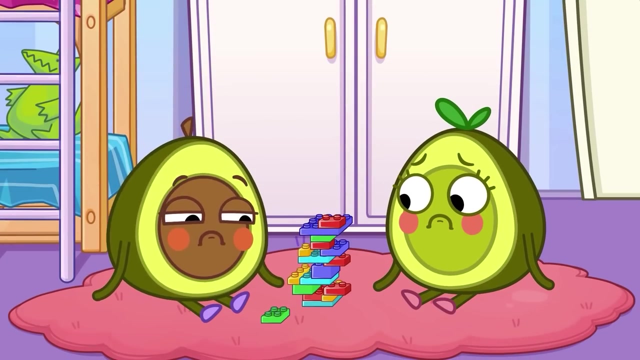 Mrs Apple will take care of the children, And she brought a treat. Mwah Bye, kids, Be good. Bye-bye Mommy and Daddy. Why don't you give Mrs Apple a chance? Pit and Penny are still sad. 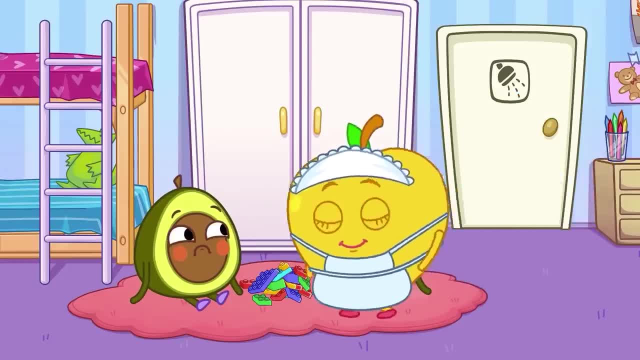 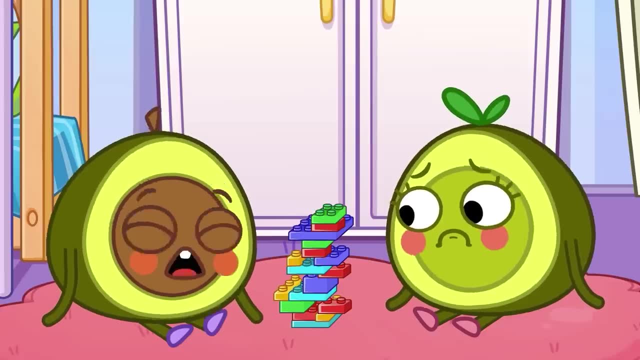 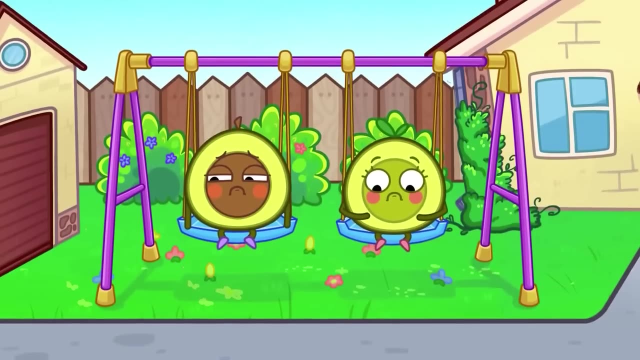 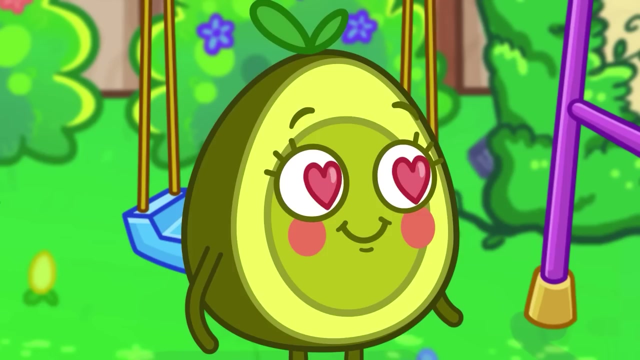 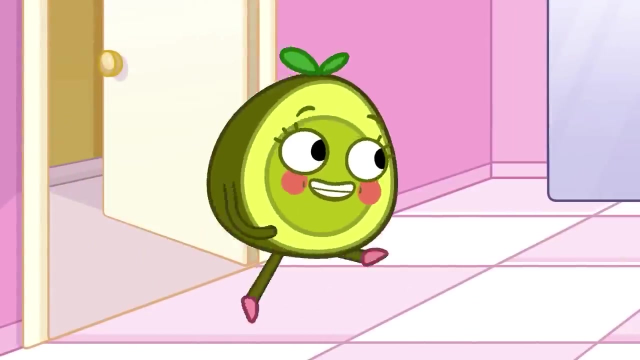 Here comes Mrs Apple, But Pit and Penny still don't want to play. Something smells yummy. Go see what it is, Penny. Good job, Ms Apple. Mrs Apple will be surprised. Have a good time. Mrs Apple baked a pie. 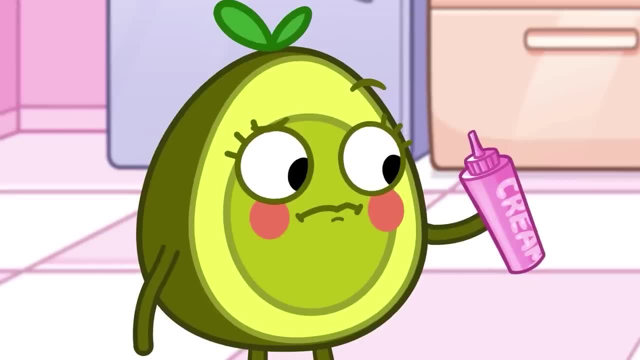 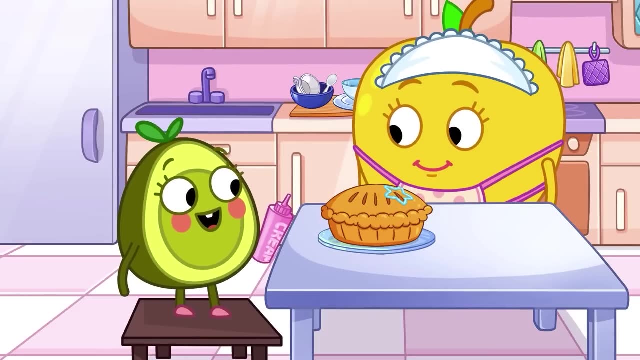 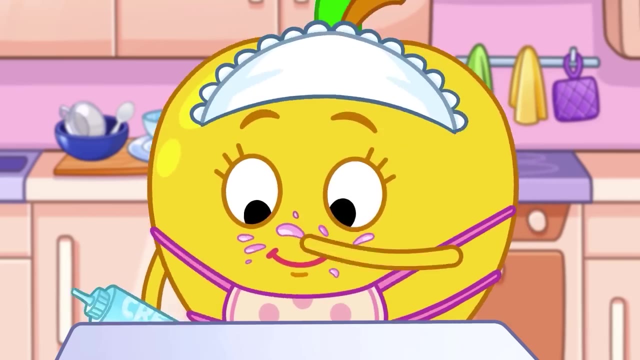 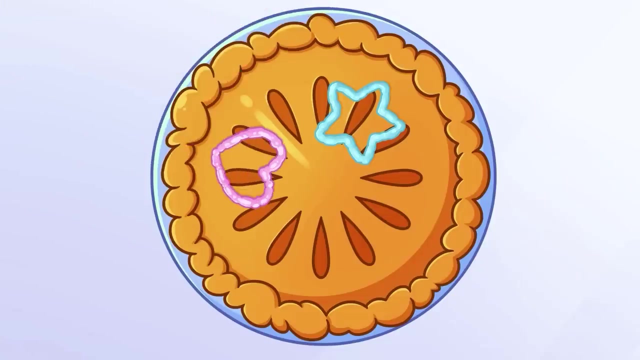 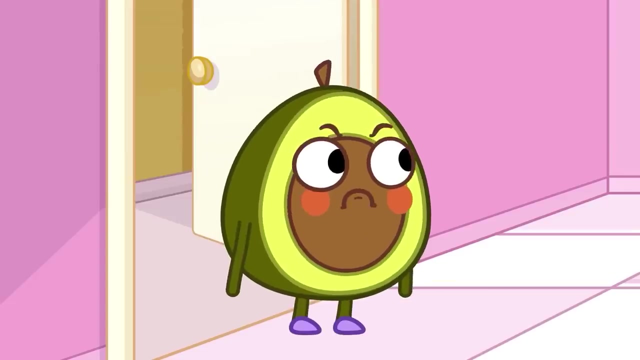 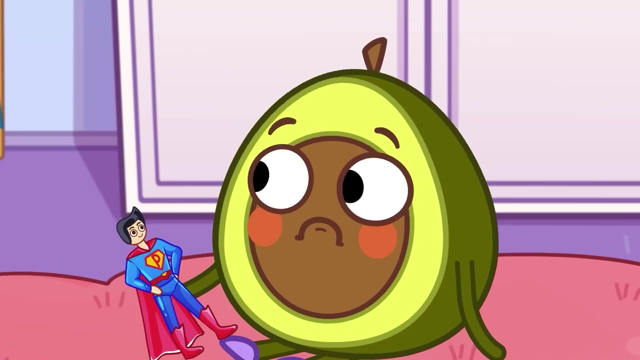 Penny can help decorate it. Oops, Are you okay, Mrs Apple? Go ahead, Penny, Try again. Penny is having fun, But Pit still wants Mommy and Daddy. Would you like some pie? Pit, He loves when Mommy brings him pie. 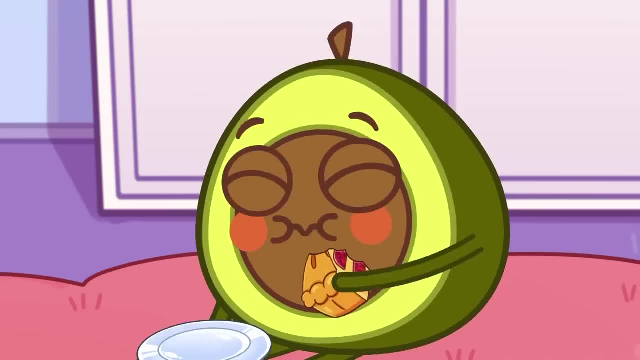 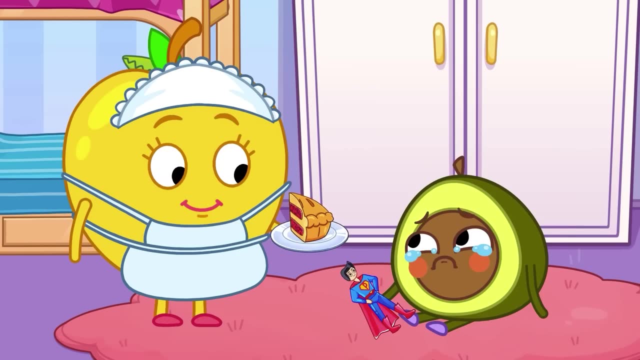 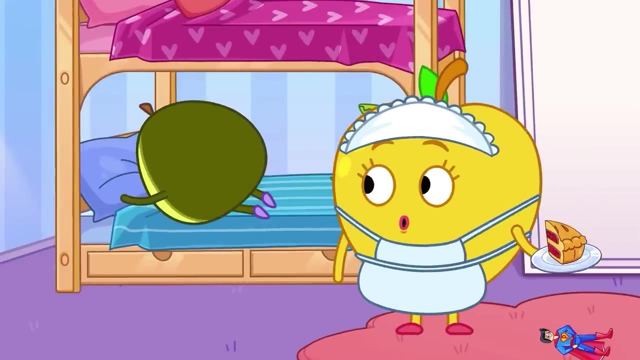 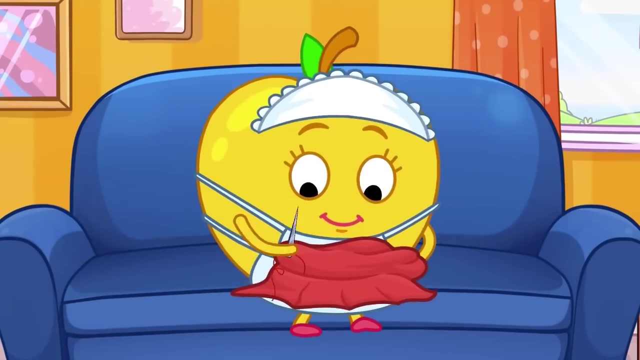 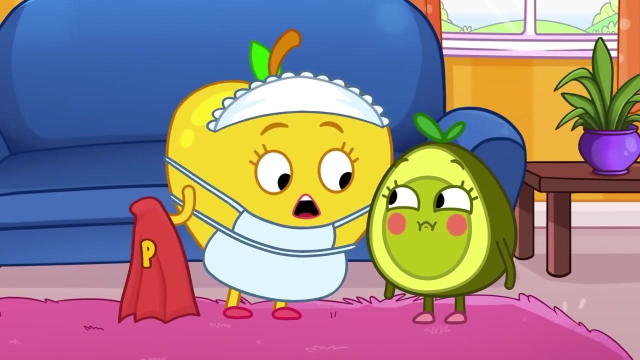 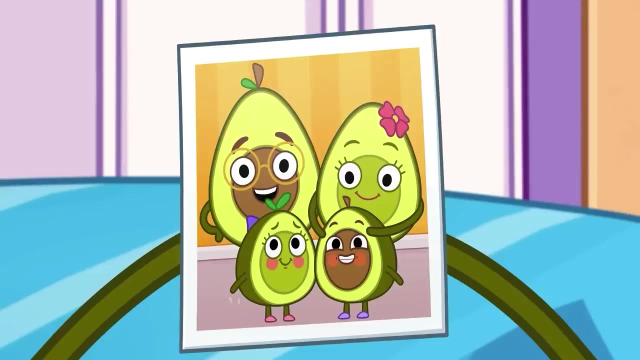 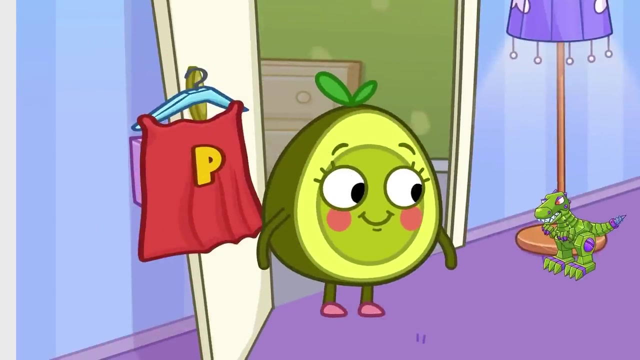 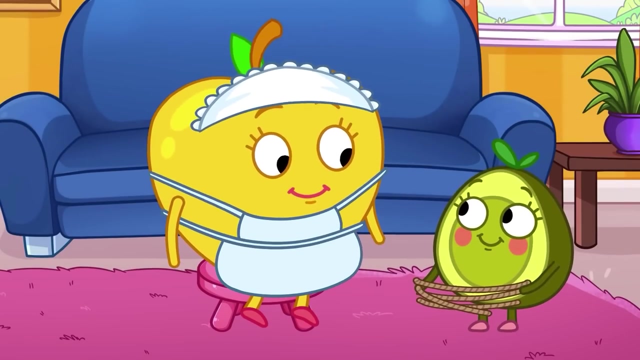 But Mrs Apple isn't Mommy. I want my Mommy back. Mrs Apple has an idea. It's a cape And a letter P. What is Pit looking at? It's a photo of his family. Mrs Apple and Penny have a plan to make Pit smile. 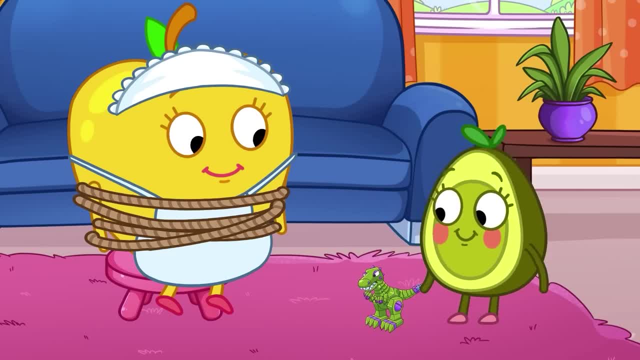 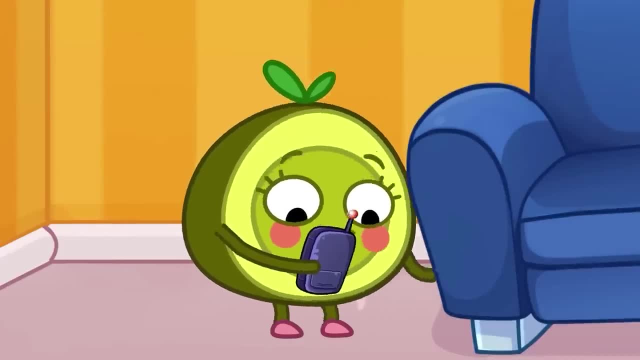 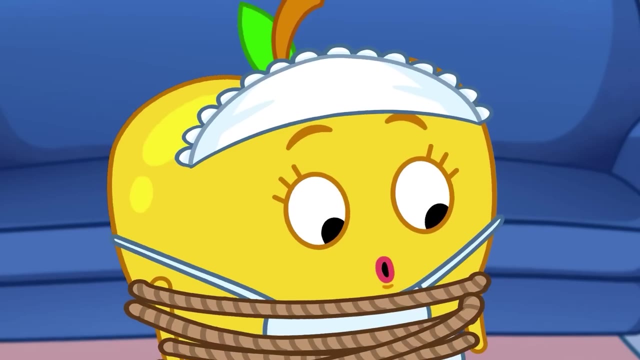 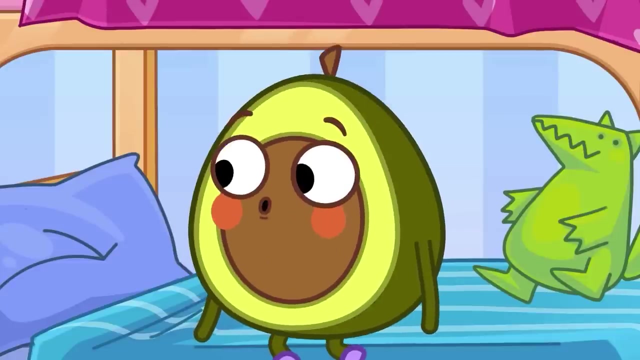 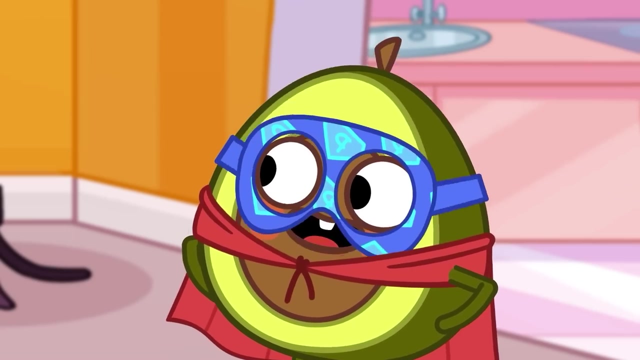 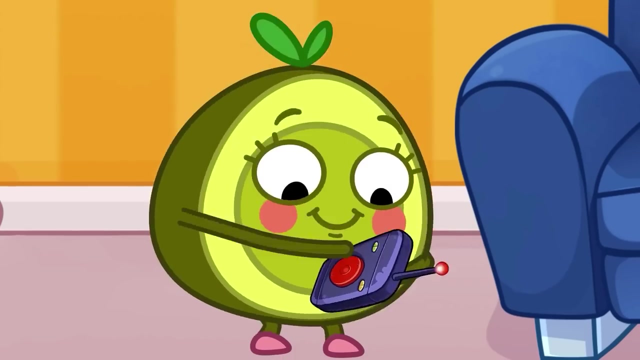 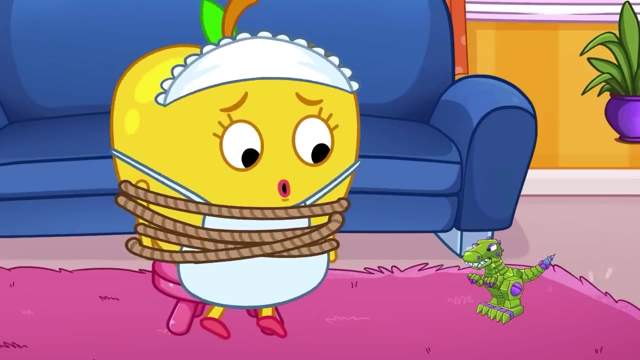 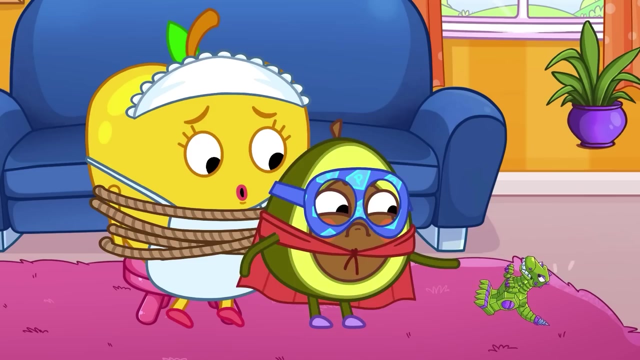 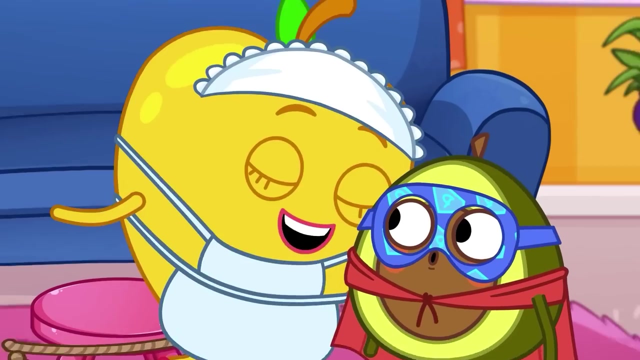 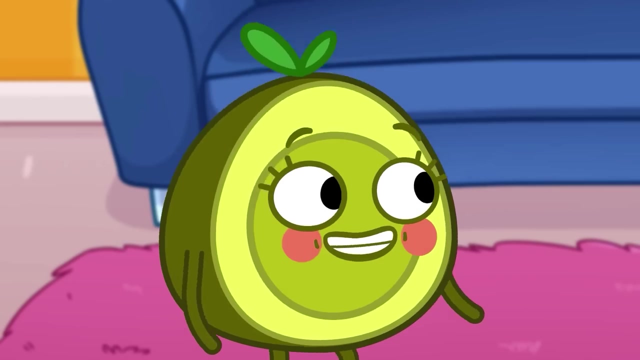 Des affirme保. Pit, someone needs you. All you need is that cape. 呢, I will save you. Hurry Pit. T-Rex is attacking. Good job, Mrs Apple is saved. You are my hero. Playing with the babysitter is lots of fun. 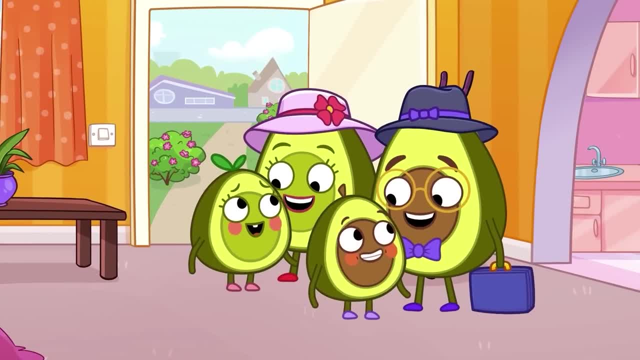 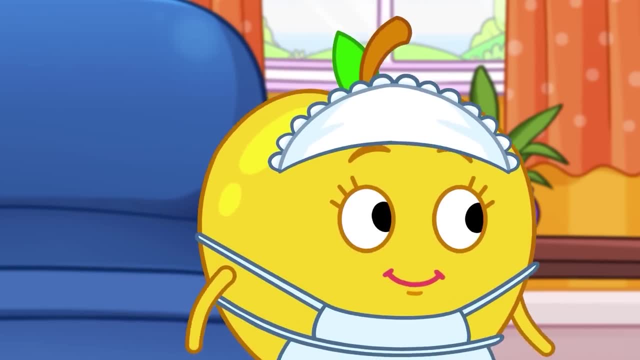 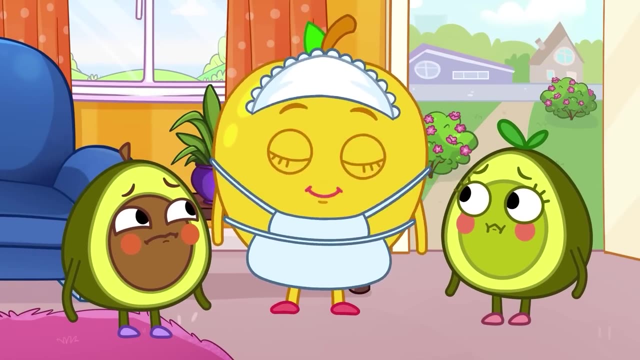 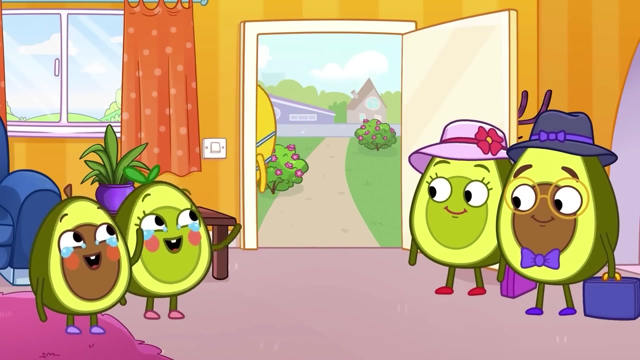 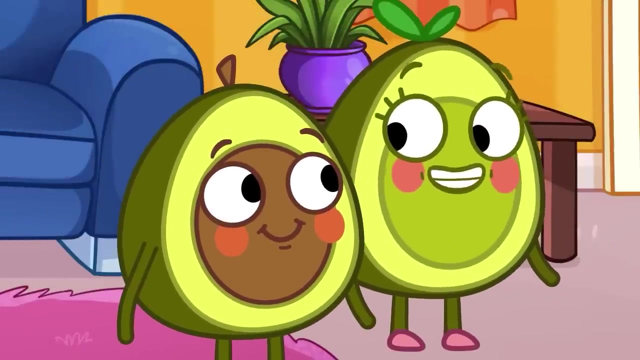 Mommy and Daddy are home. It's time for Mrs Apple to go. Please don't leave. It's okay, kids See you tomorrow. Yay, She'll be back. Bye, Our babysitter is awesome. Pit and Penny are playing outside. 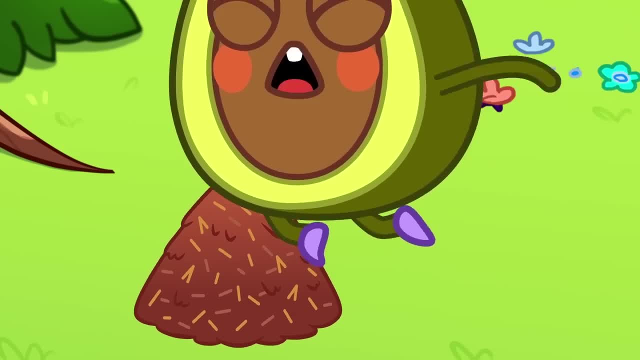 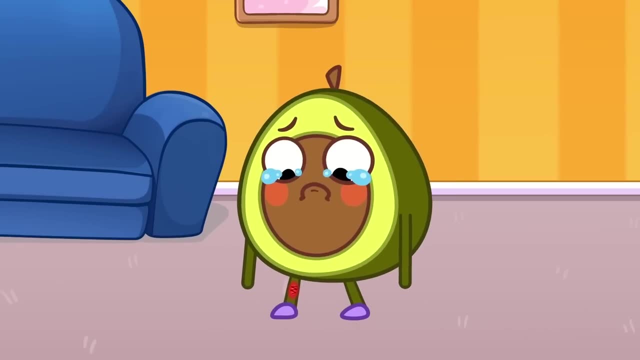 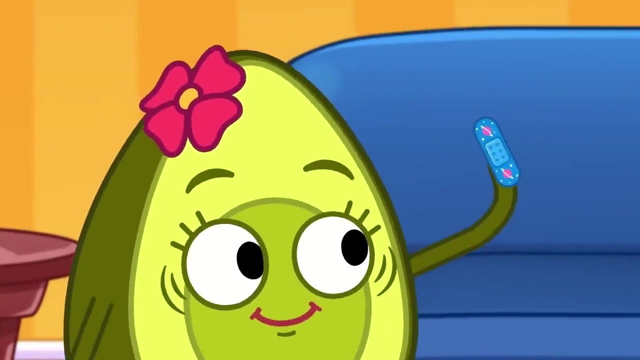 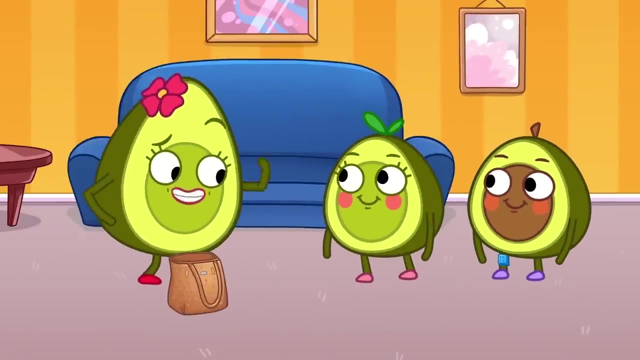 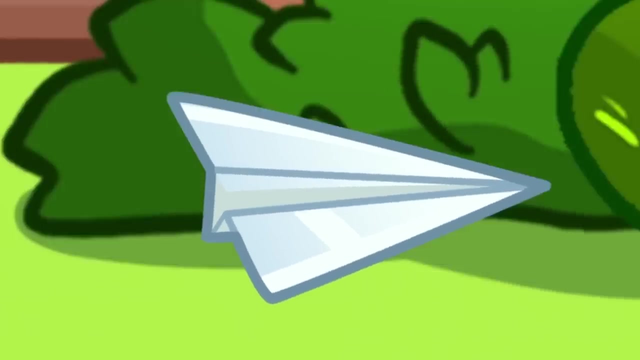 Look out, Pit Pit has fallen down. Pit Pit has hurt his leg. Mommy knows how to make this better. She has a band-aid. How does that feel, Pit? That's it, Pit. Watch where you're playing. 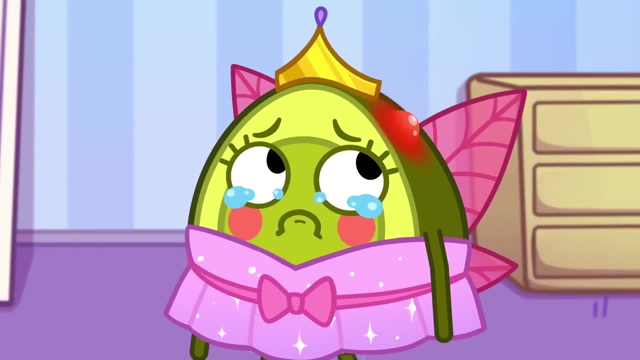 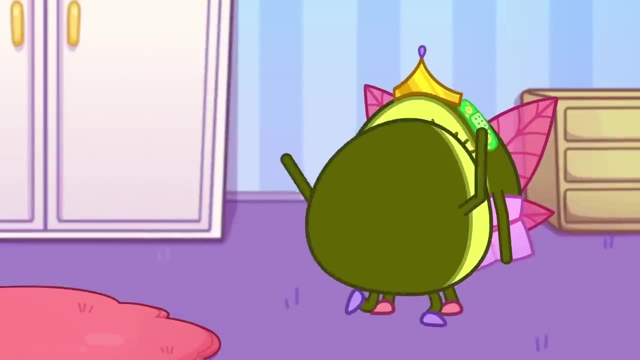 It's time for her to go to bed. Penny has had an accident. That's how you play. Don't cry, Penny, Ugh Ha. Look, Daddy has a band-aid too. Pit will help put it on. Be careful. 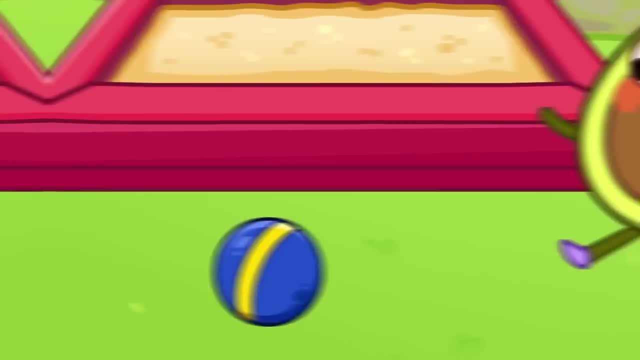 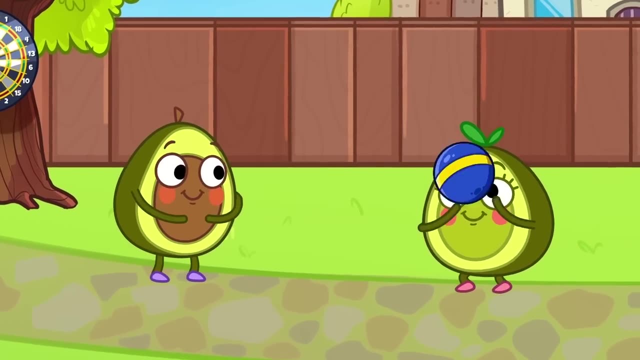 That's good. that's good. That's a good idea. Pit, Pick up your toys. Hit the music, want some? Pit and Penny are playing catch. Pit and Penny are playing catch. You can play with all of you. Hit the music, want some? 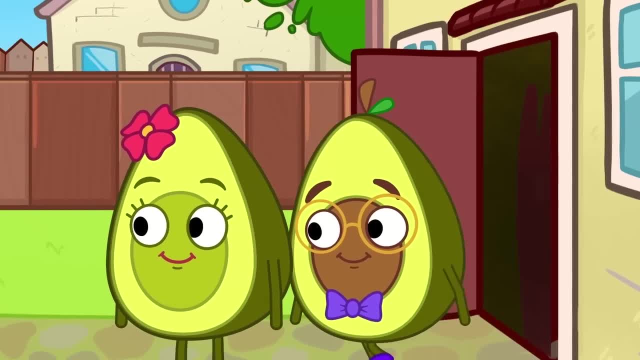 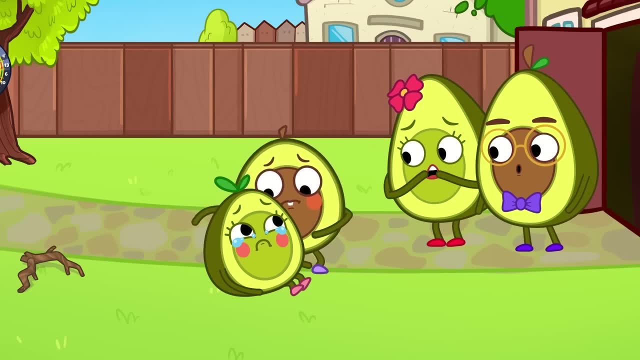 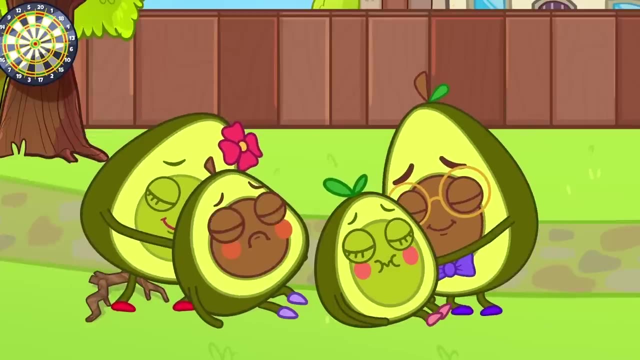 This will help you play Hit the music. want some Hit the music, want some. That was too hard Pit, It was fun Hit the music. want some Hit the music? want some Pit? watch out, honey is falling down again and the ball has hit pit, I think. 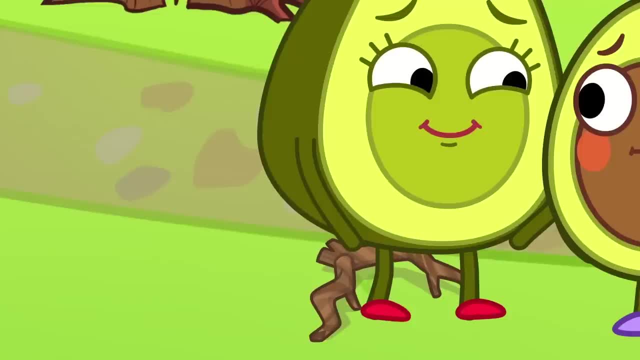 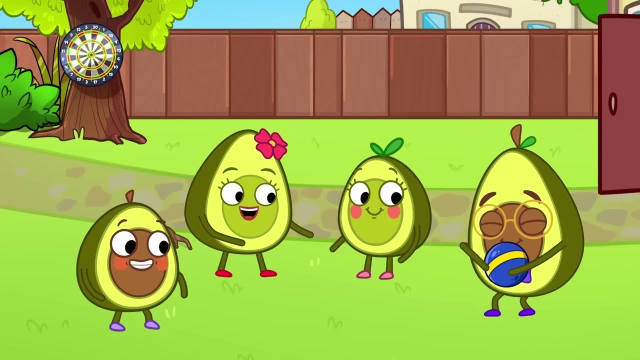 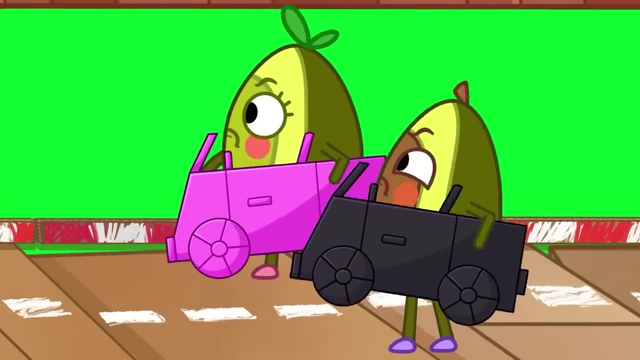 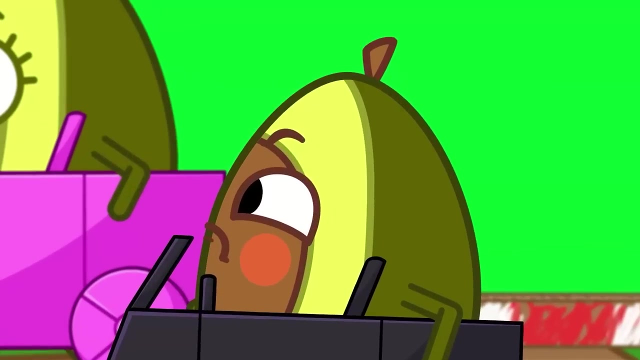 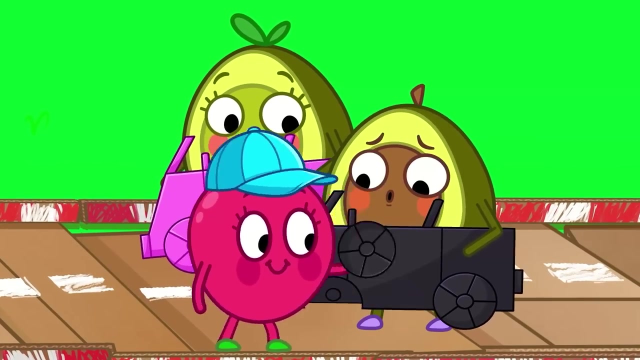 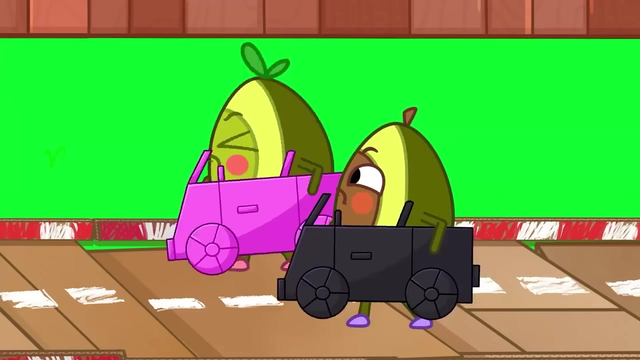 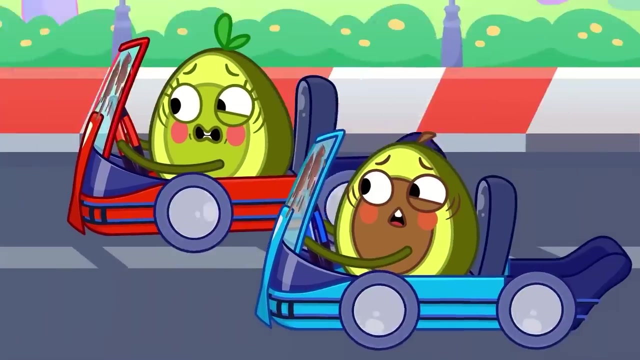 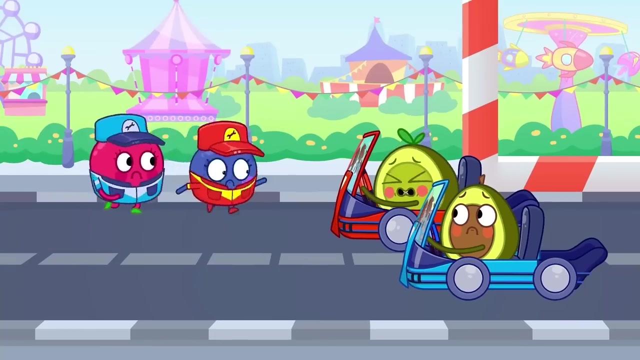 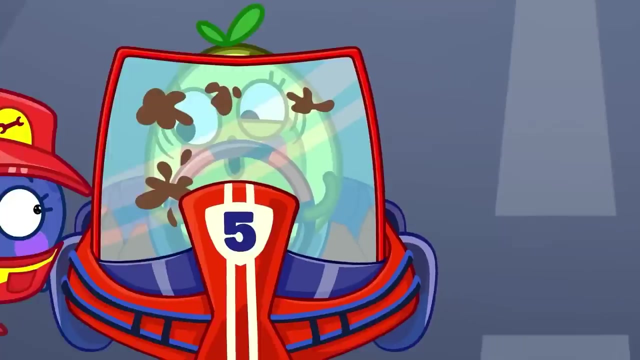 you both need a hug. be careful. mommy has an idea. everyone is playing catch and having fun. hit and penny are ready for a race. hey, your tire came off. don't worry, cherry will fix it and they're off. oh no, they got mud on their windows. hurry pit crew, the kids need you. cherry gets this window nice and clean. 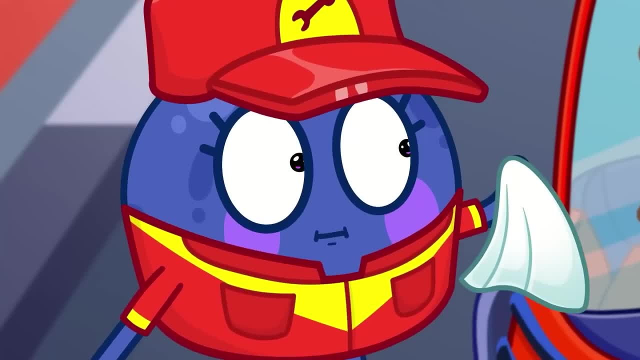 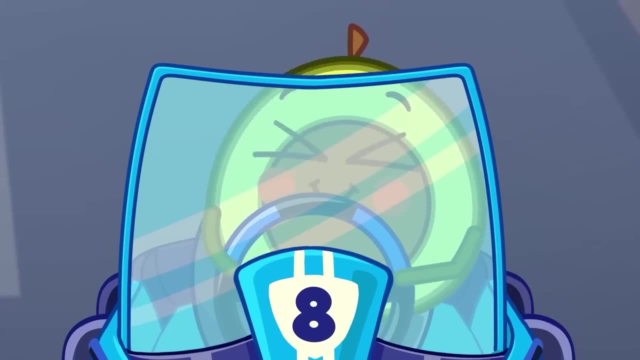 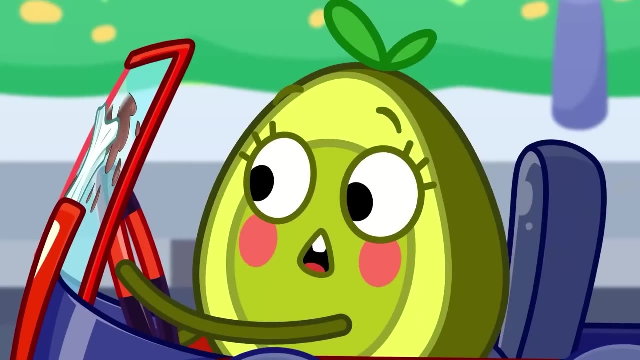 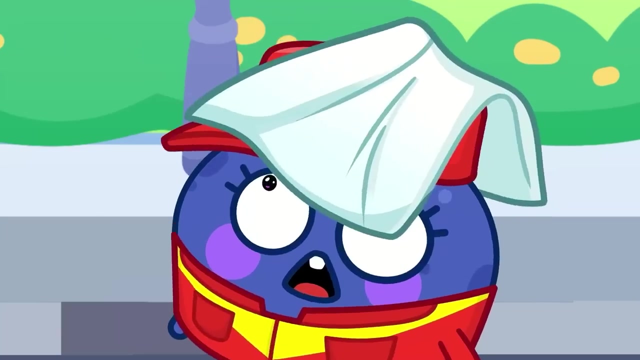 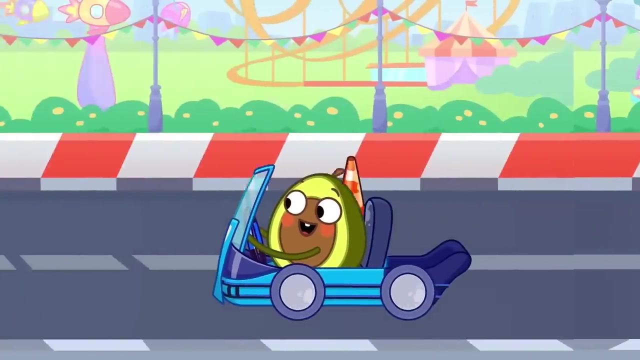 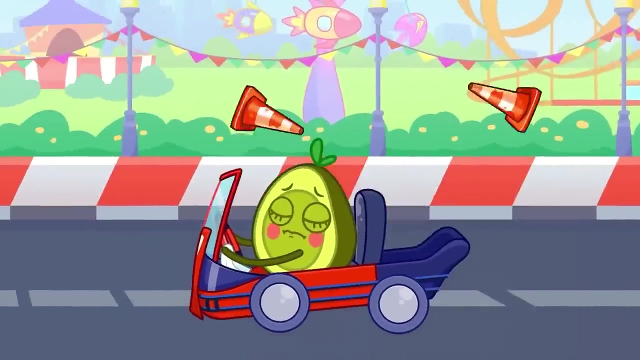 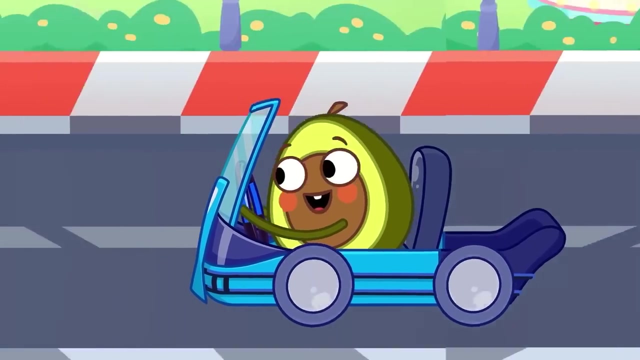 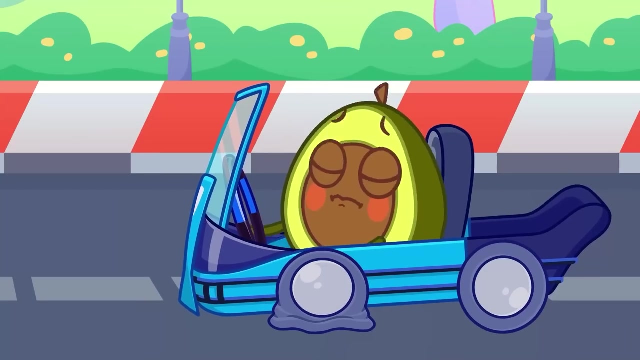 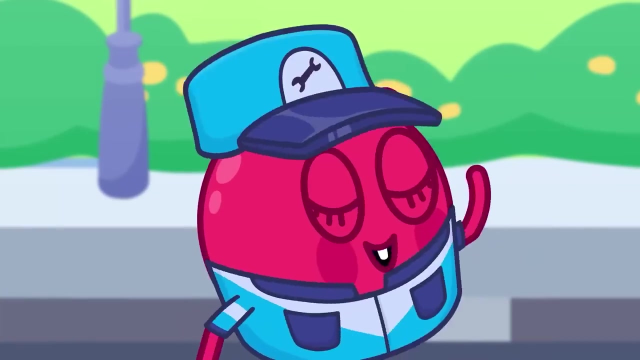 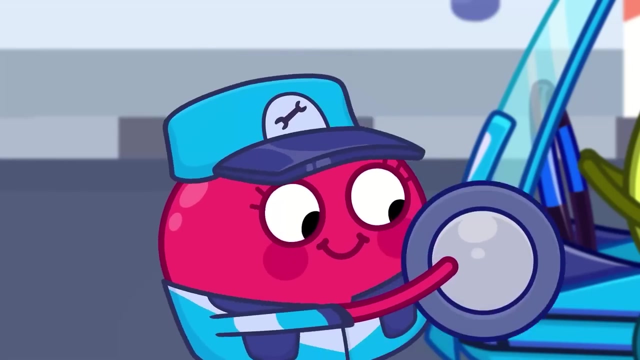 but blueberry makes pennies window worse. oh, oh, oh, oh oh, it is in the lead patty, catch up, not with a flat tire. watch, the road pit pit has a flat tire too. cherry will put on a new tire. oh, oh, oh, oh, oh, oh oh. 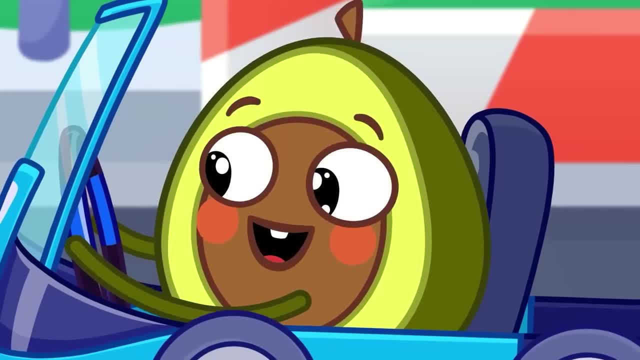 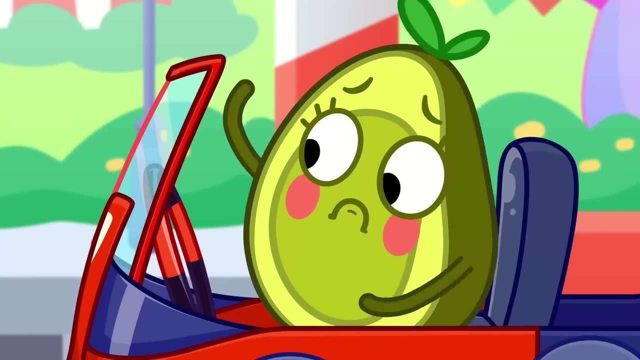 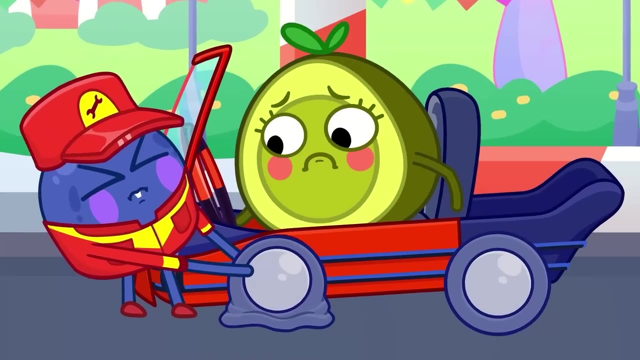 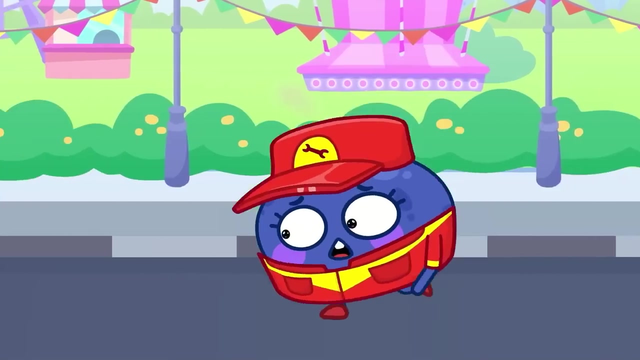 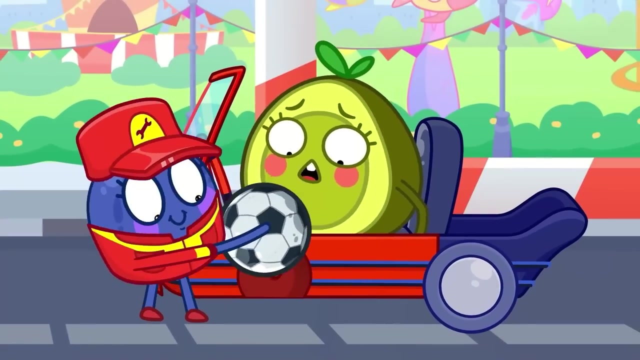 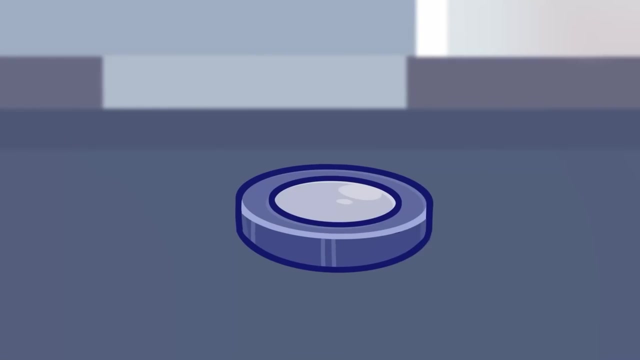 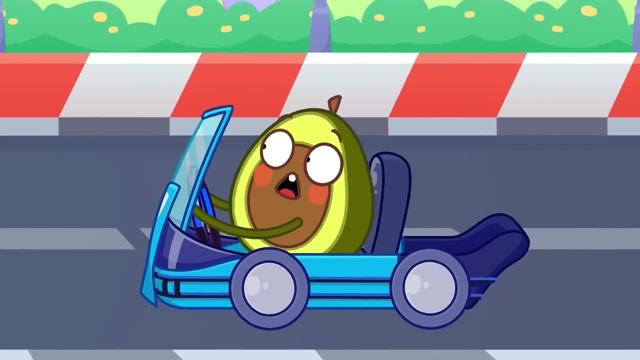 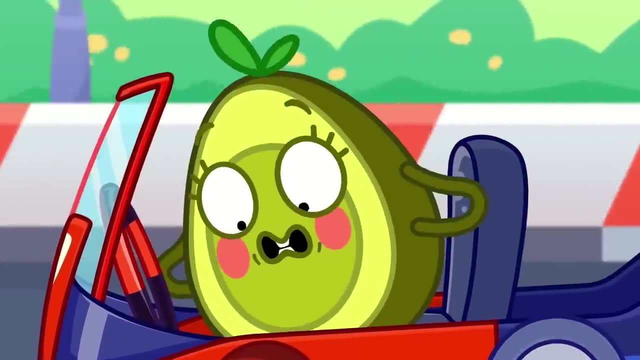 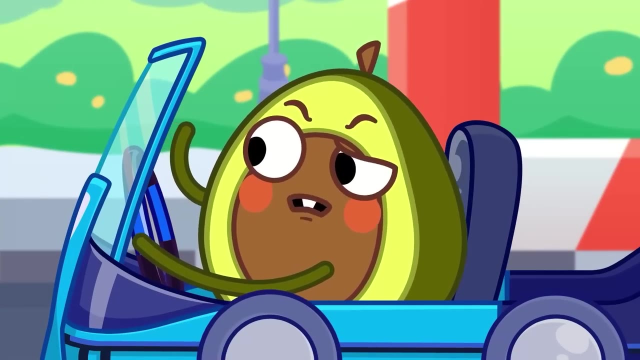 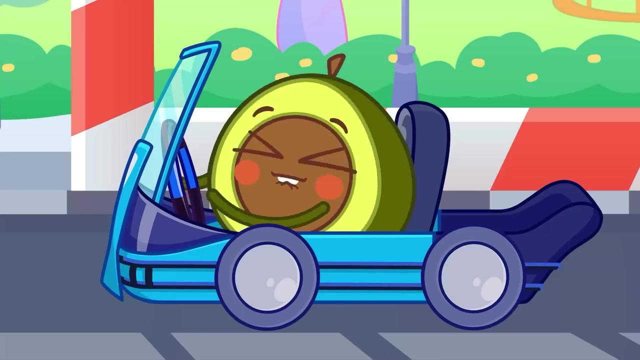 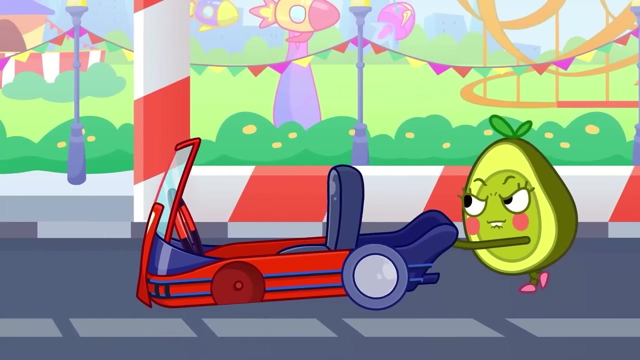 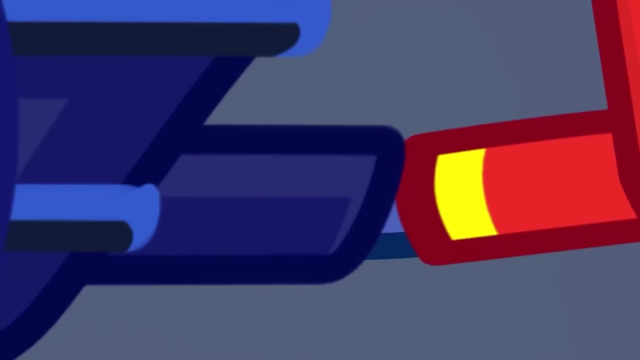 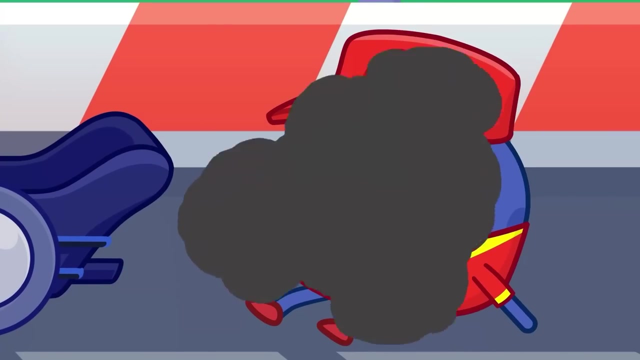 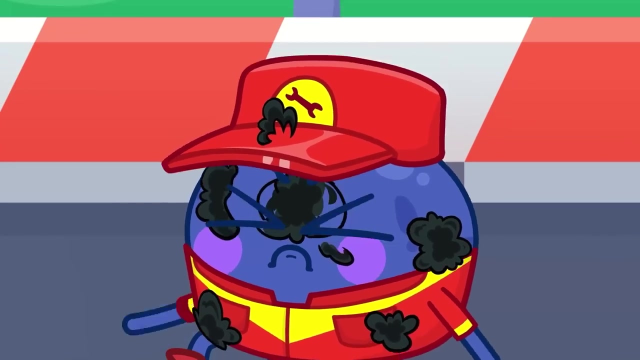 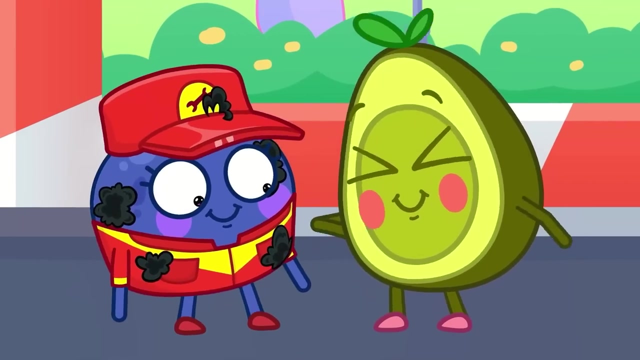 Pit is out of fuel And the soccer ball popped. Make my car faster. The car just needs some gas. Blueberry's hand is stuck. Oh, I can do anything. Don't cry. Blueberry Penny is here to help. 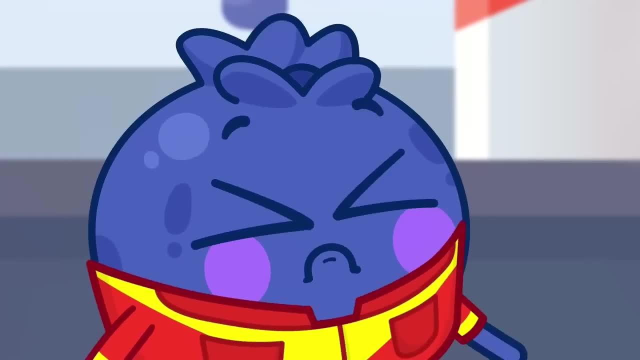 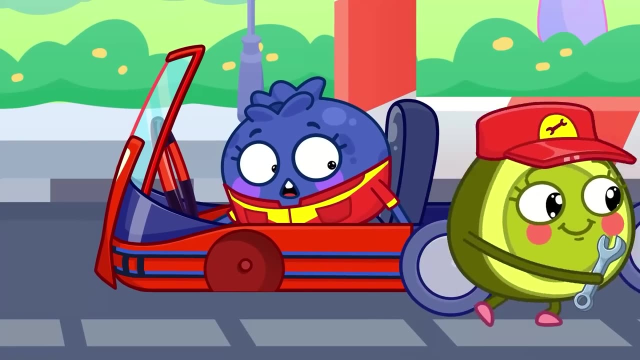 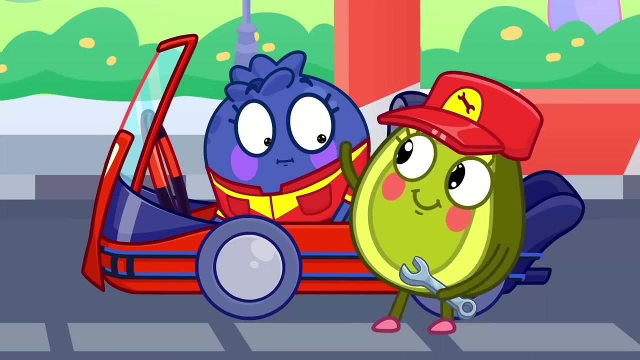 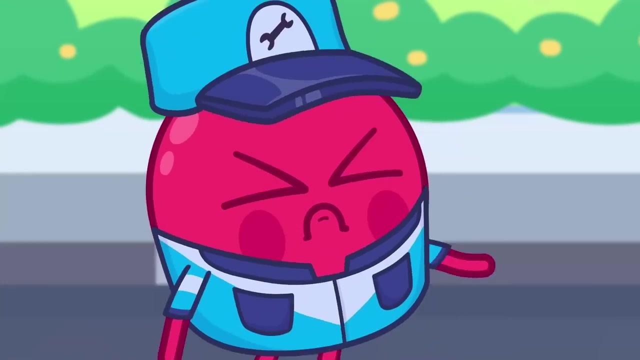 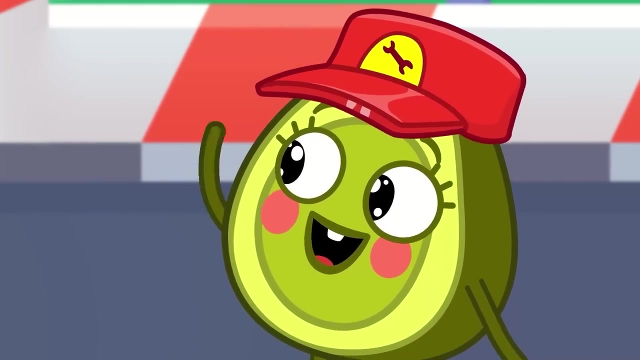 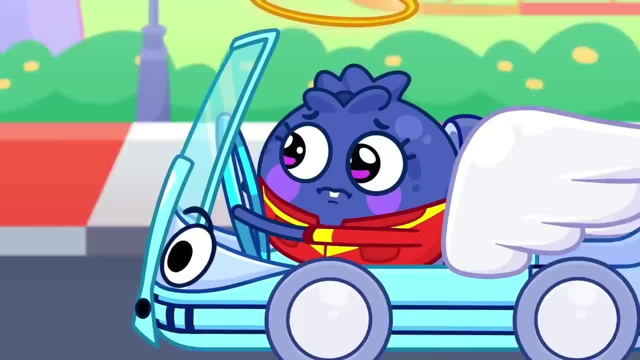 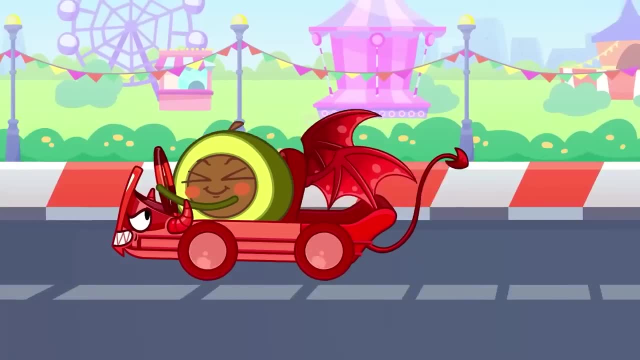 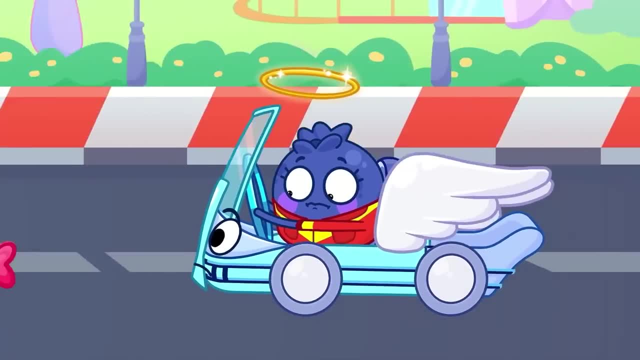 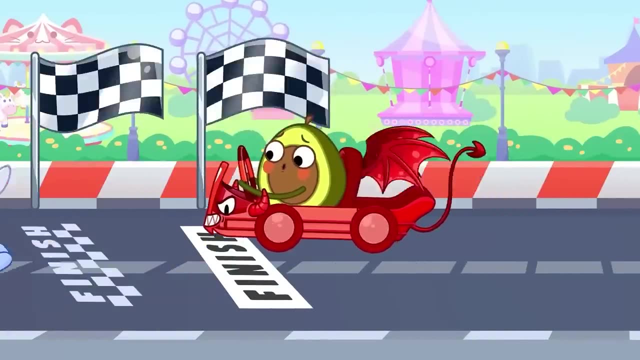 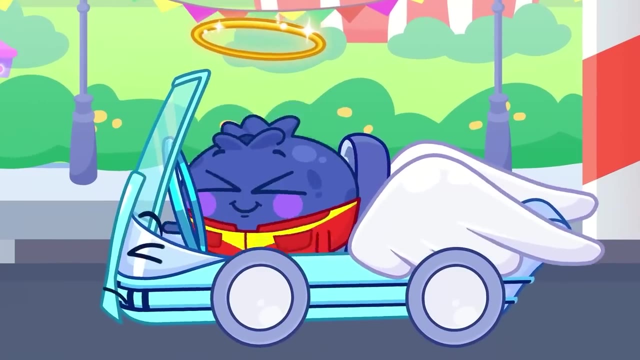 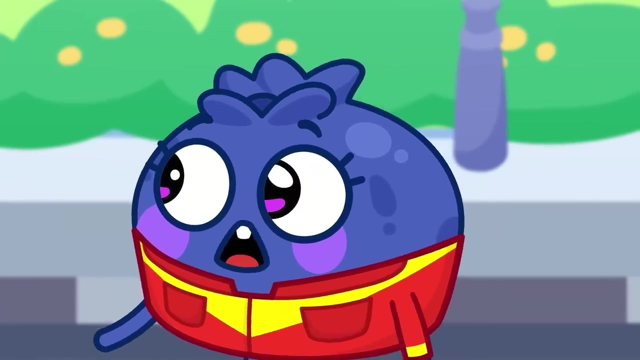 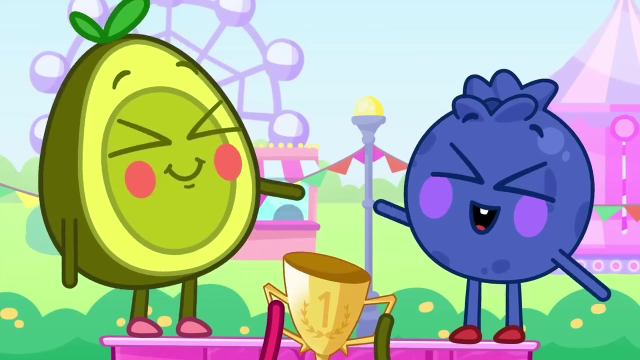 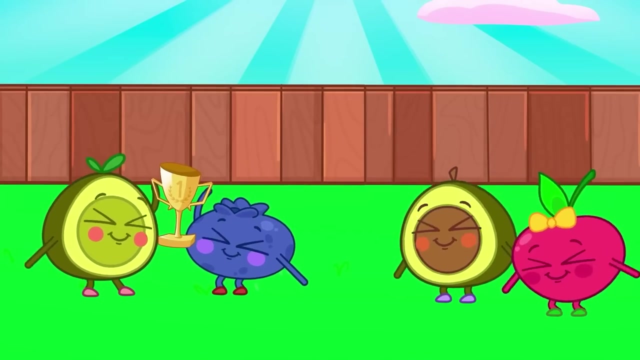 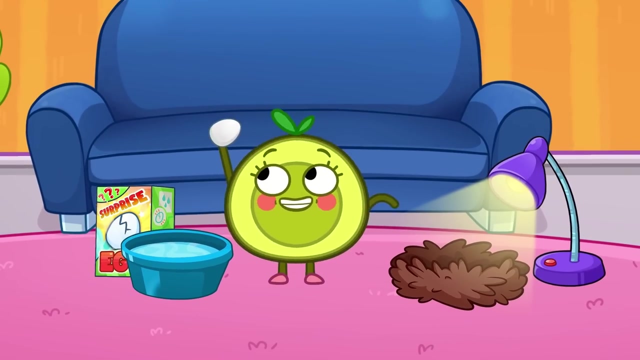 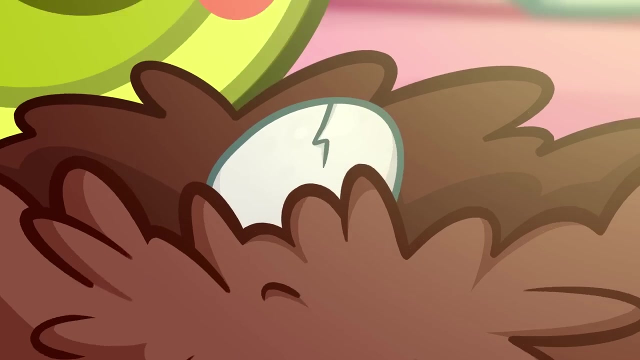 Watch out for the wall. Blueberry wins the race. We have won, And here's your trophy. You did it by working together. Penny has a new toy. It's an egg with a surprise inside. Look, It's starting to hatch. 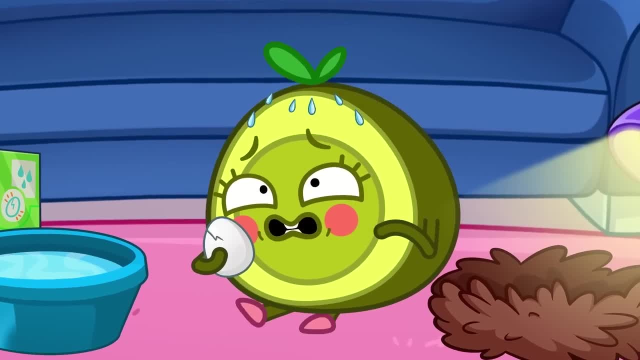 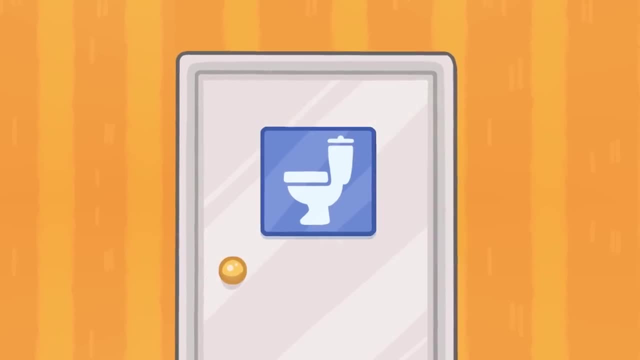 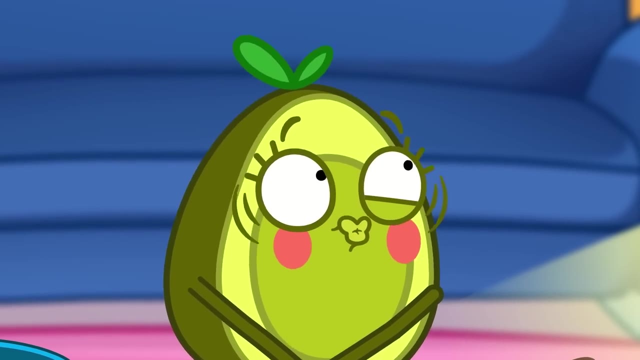 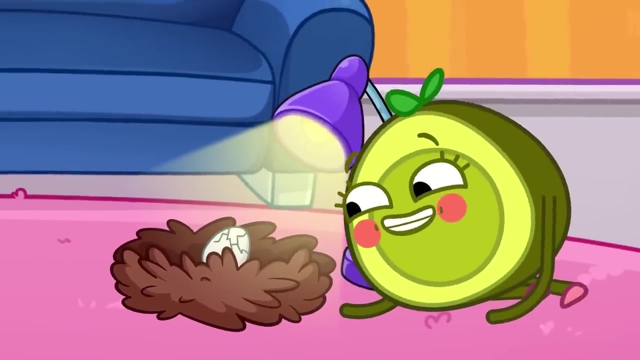 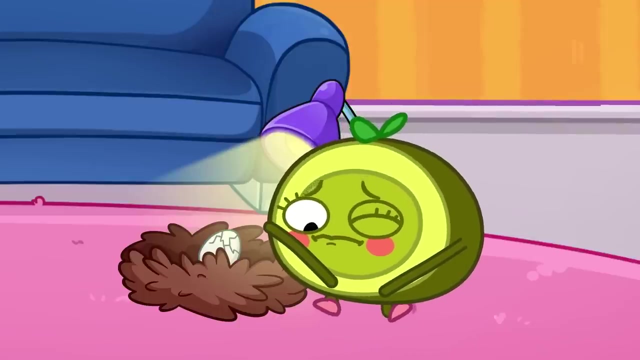 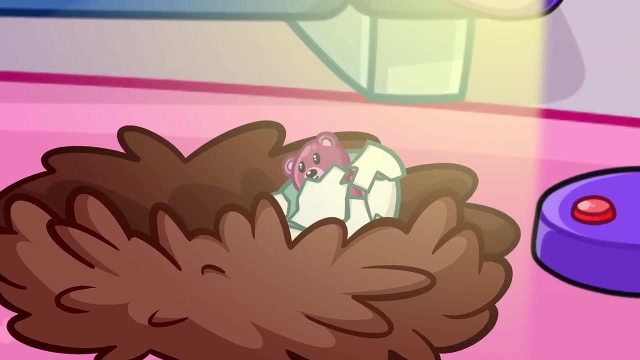 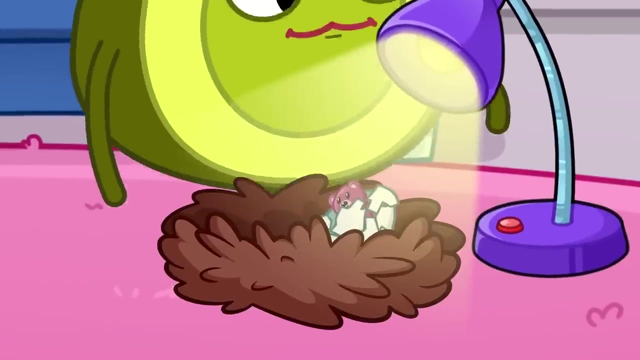 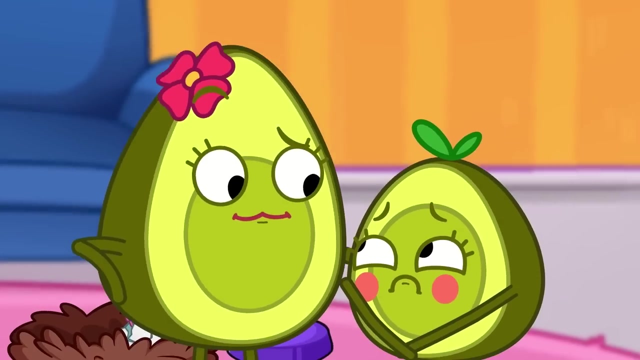 Penny needs to use the potty. Don't hold it in. Penny, Go to the bathroom. She doesn't want to miss her surprise. Mommy, can you help Now? the surprise can wait, Penny, it's time to go to the toilet. 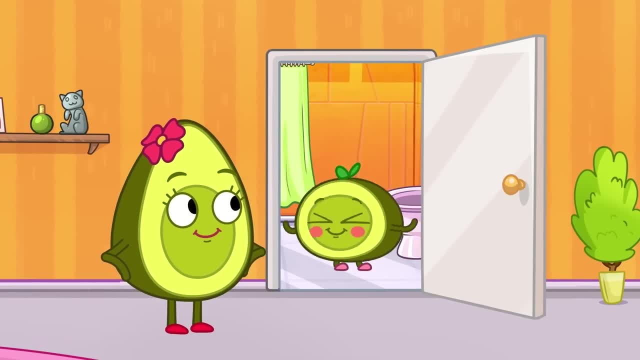 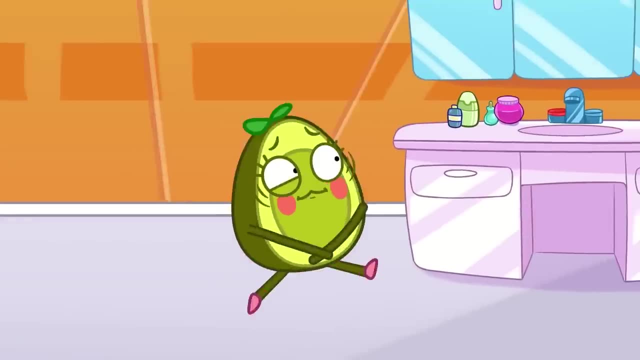 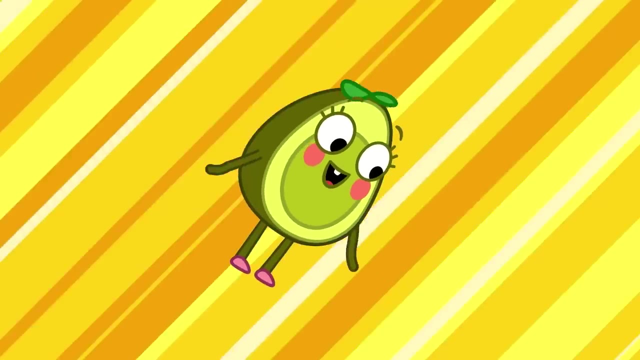 You'll feel much better when you're done. To the potty, To the potty, Have a seat. To the potty, To the potty, P-P-P. To the potty, To the potty, Have a seat. 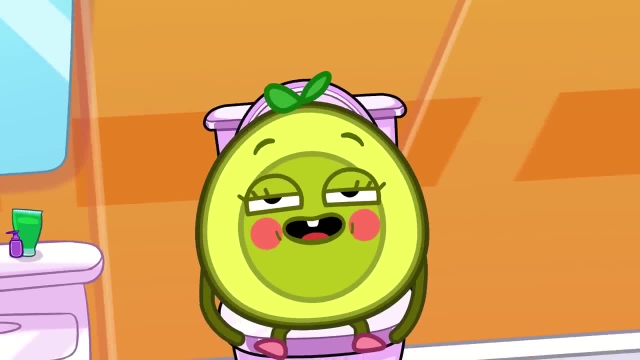 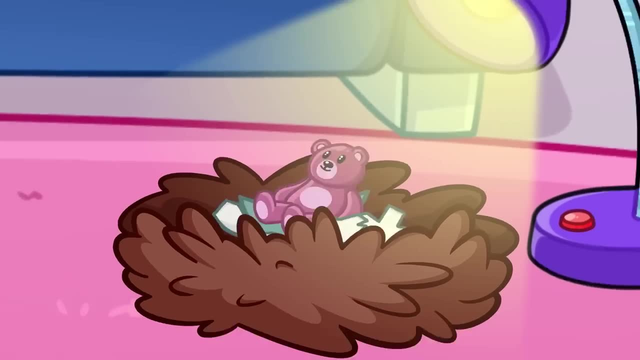 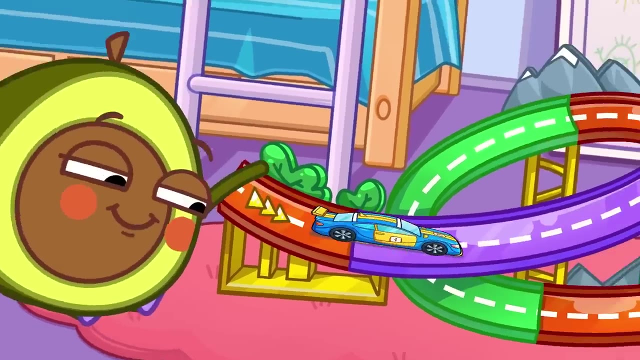 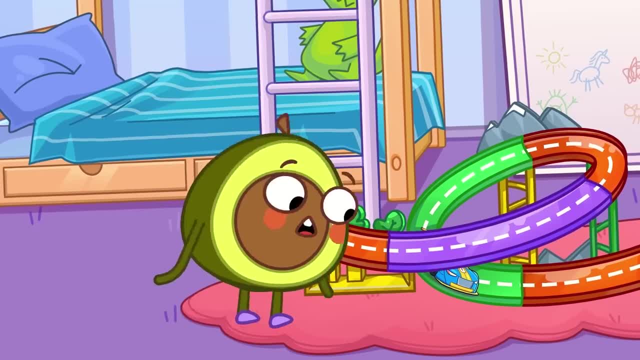 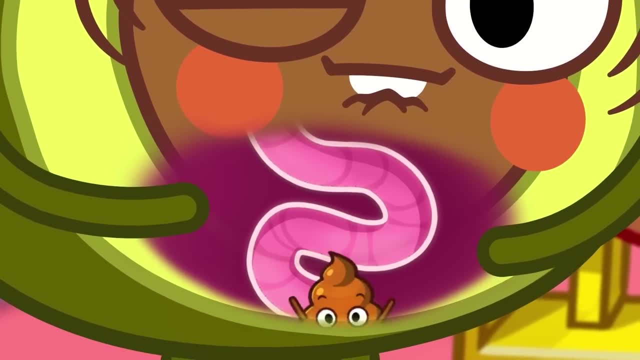 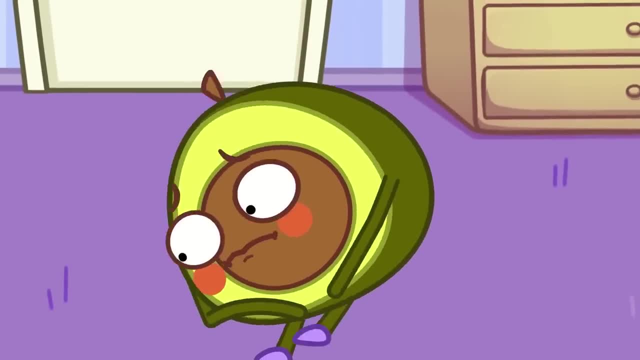 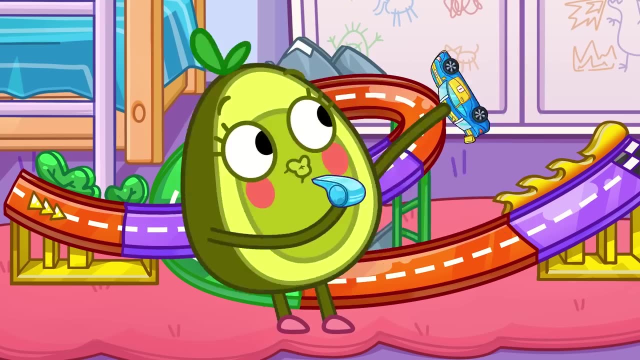 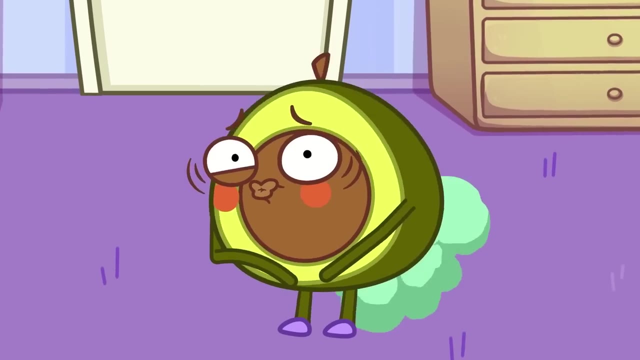 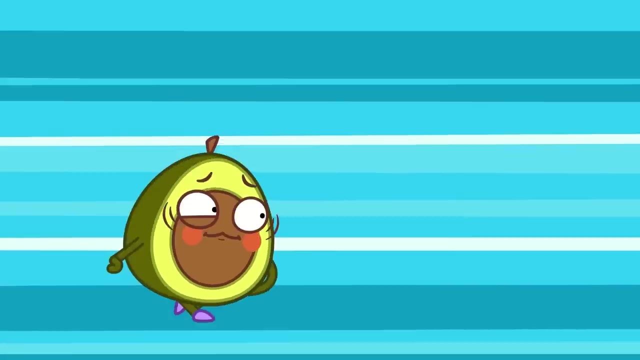 But he wants to watch his car jump. Penny has something to say: Pit, don't keep it in, Better go to the toilet. Hurry Pit To the potty, to the potty. I have a seat. To the potty, to the potty. I puk my teeth. 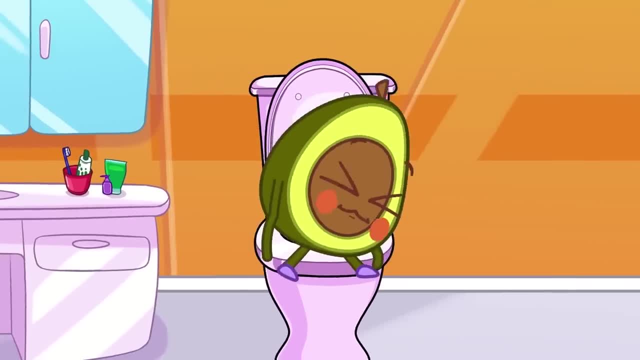 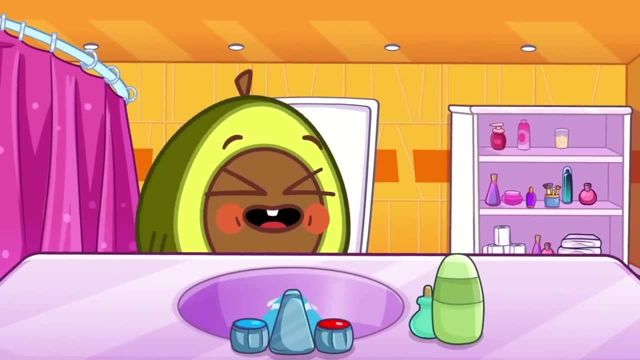 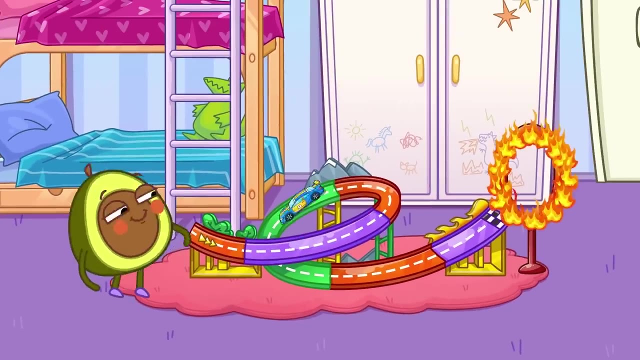 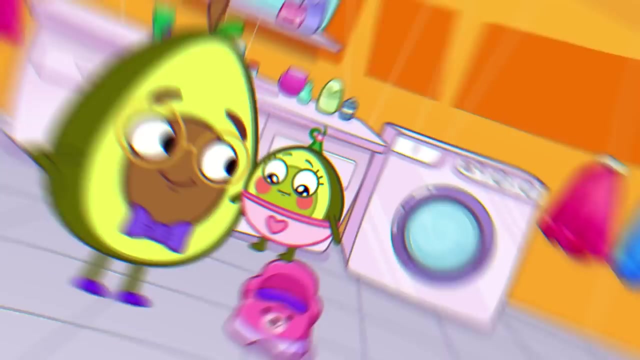 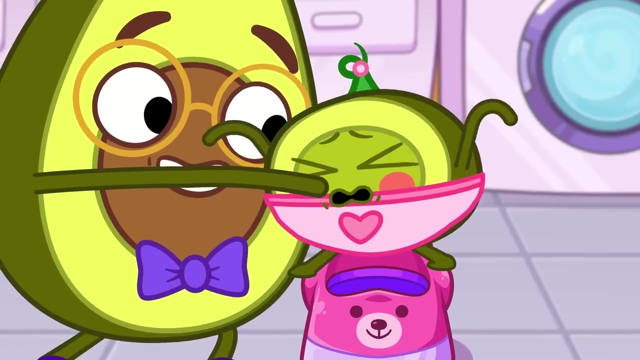 To the potty. to the potty, I have a seat To the potty. to the potty, I puke my teeth. Now Pip feels much better. Daddy is teaching Baby how to use the potty, But Baby doesn't want to use the potty. 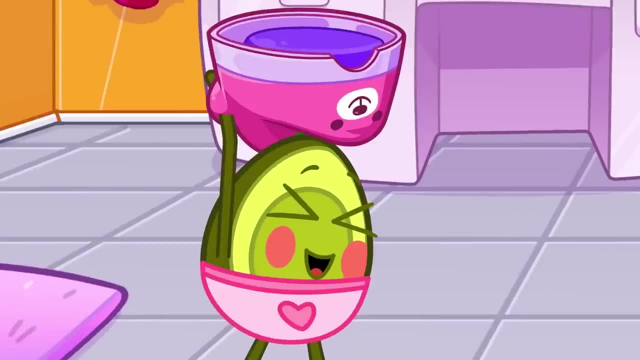 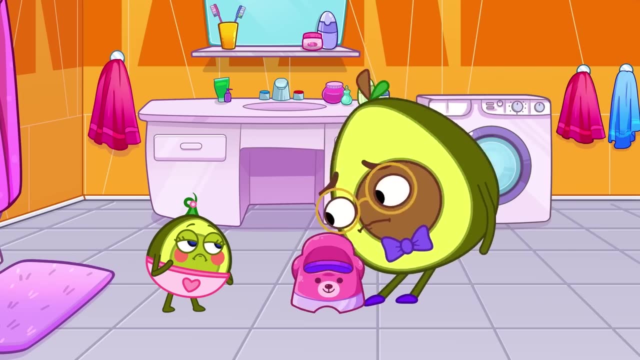 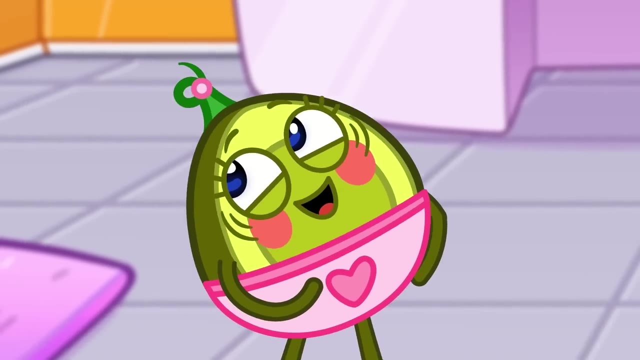 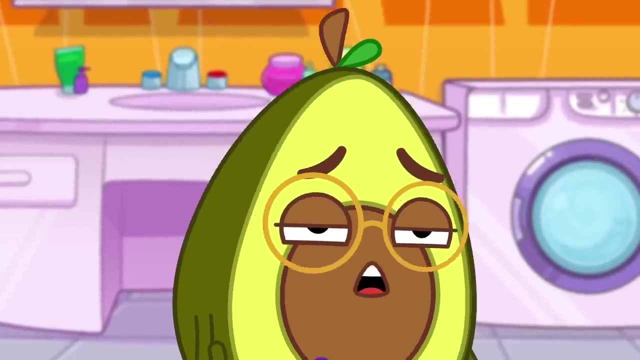 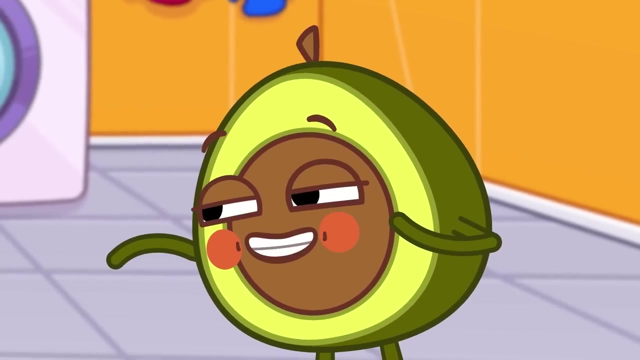 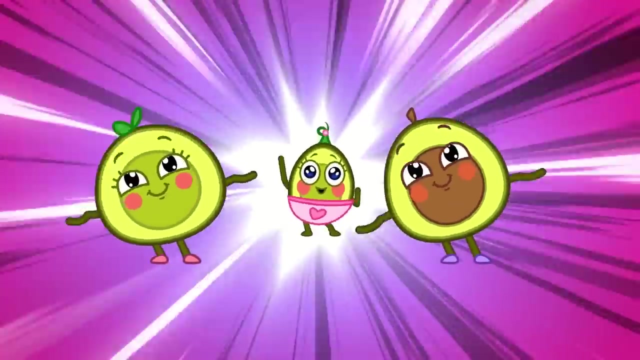 No, Baby, it's not a hat. Maybe Daddy should show her. Oh, now the potty's stuck. Dad, We will help you. Let's all sing the potty song To the potty, to the potty, I have a seat. 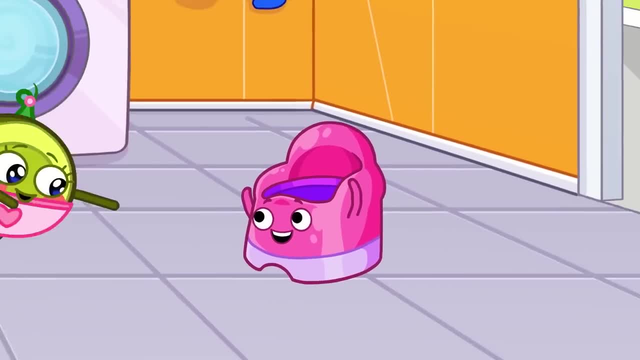 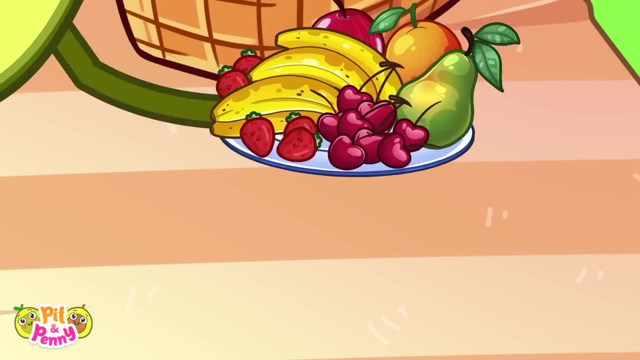 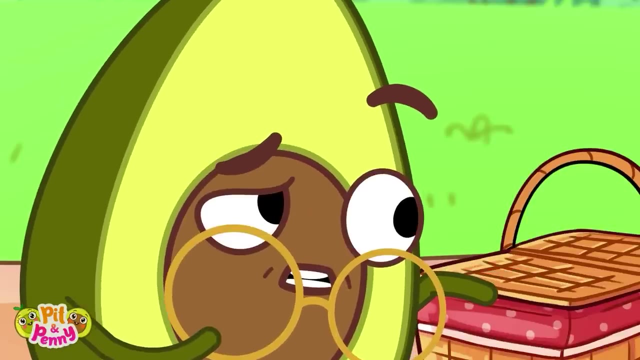 To the potty. to the potty, I have a seat. It worked. Yay, What a lovely day for a picnic. Daddy brought fruit and sandwiches. Here come Mommy and Penny. Penny is wearing a flower, But Mommy doesn't have one. 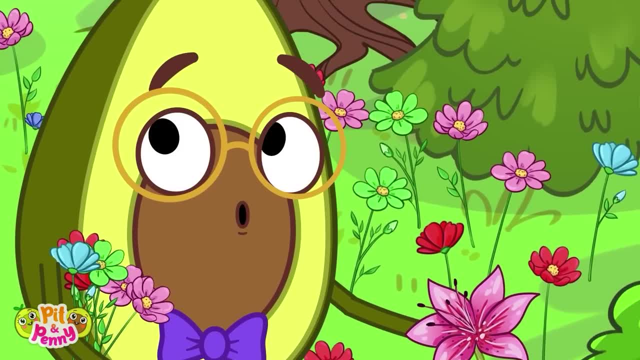 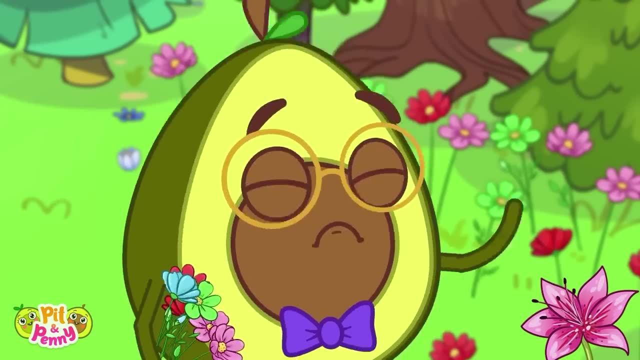 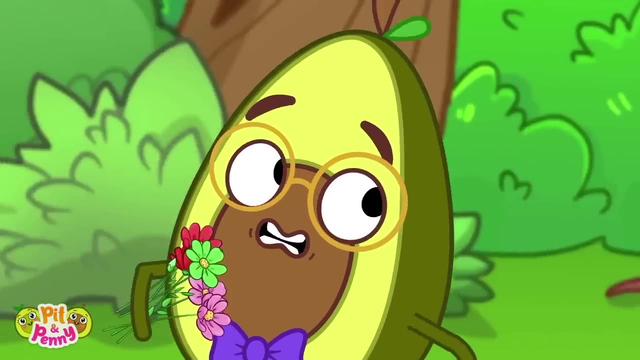 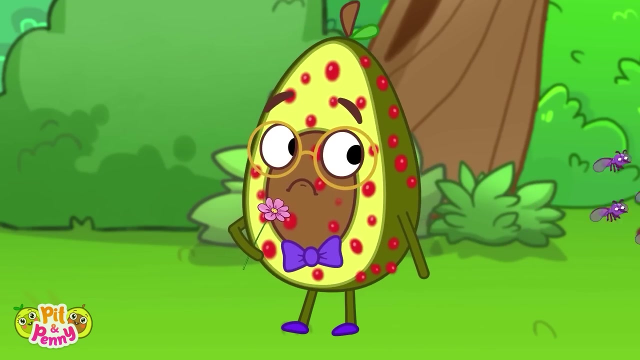 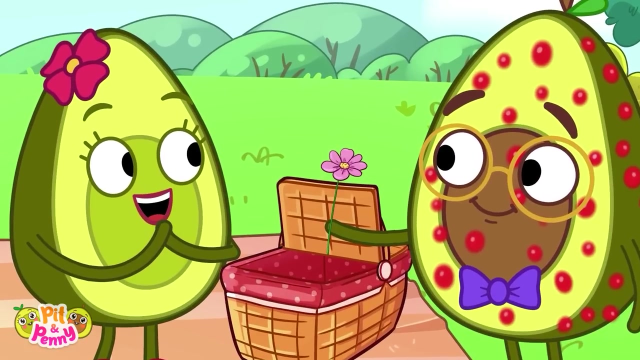 Oh, pick that flower for Mommy. What's that sound? It's a mosquito. Hurry, it might bite you. Daddy made it. Oh, no More mosquitoes, And poor Daddy's been bitten all over. Mommy, can you help with Daddy's mosquito bites? 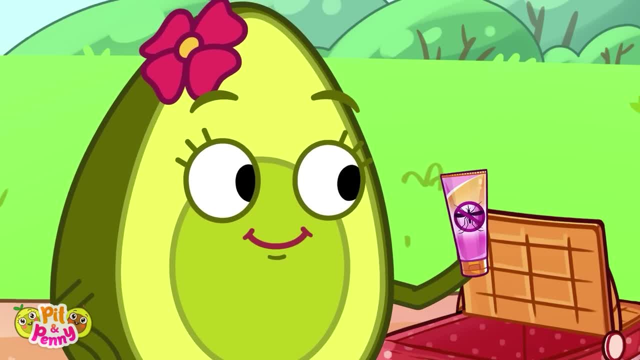 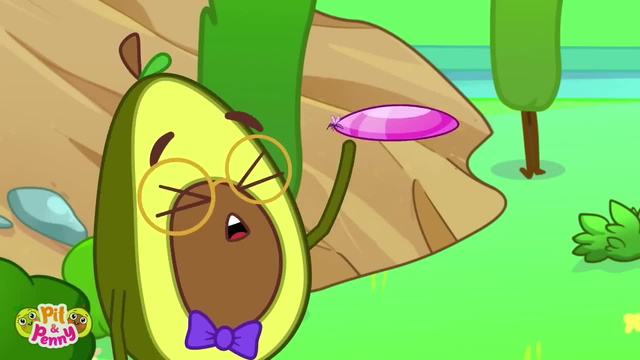 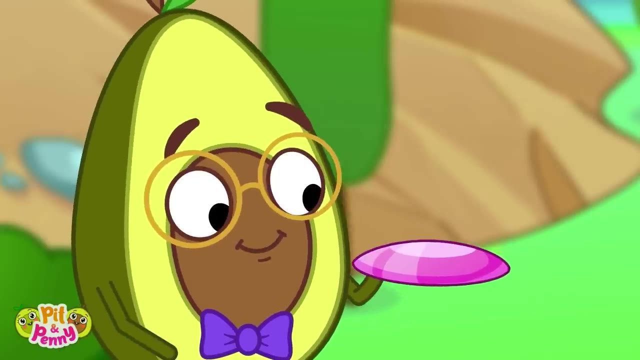 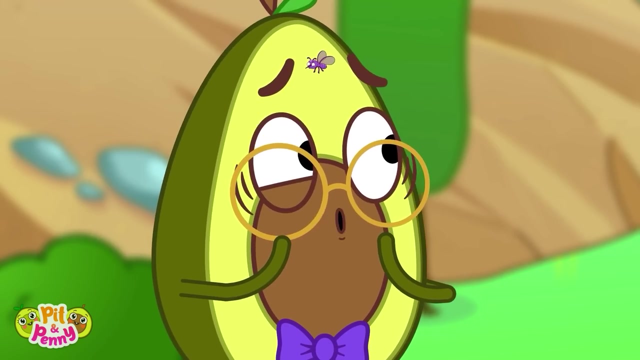 Honey, don't forget the bite bomb. It makes bug bites less itchy. It's time for a game of frisbee. Someone help. Penny blew the bug away. Now it's on. Daddy Pit. Penny, Do something, Ugh. 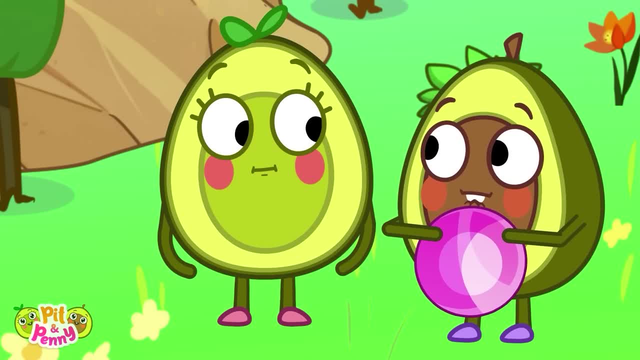 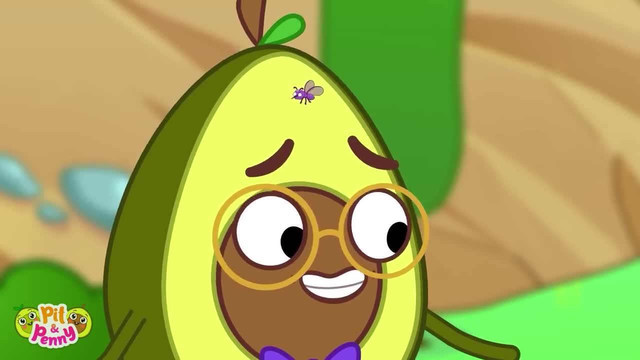 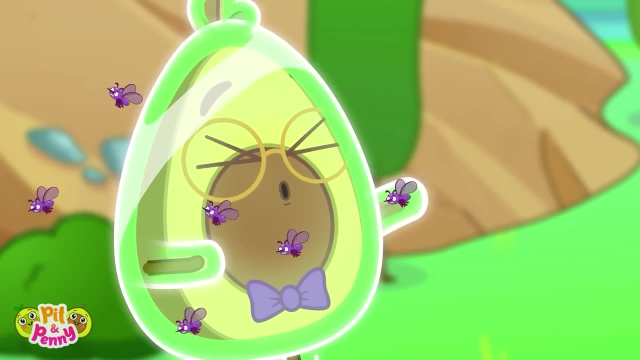 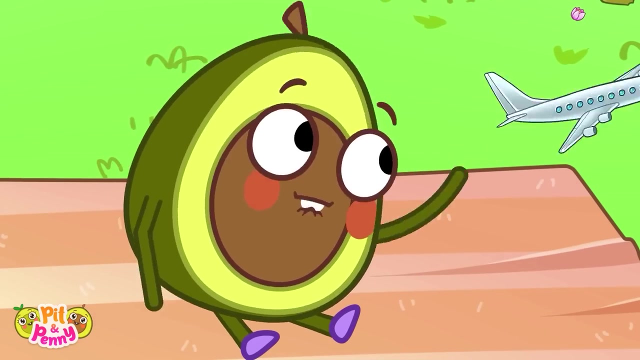 No Pit Throwing. something would hurt Daddy. Penny has an idea. Penny has an idea: She'll use bug spray. She'll use bug spray. Now, the mosquitoes can't bug, Daddy. Hahaha. What's wrong, Penny? It's a mosquito bite. 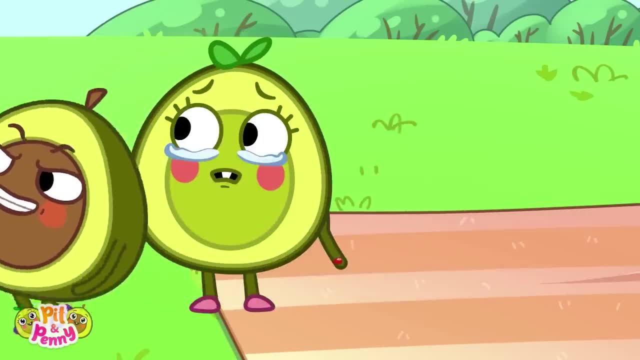 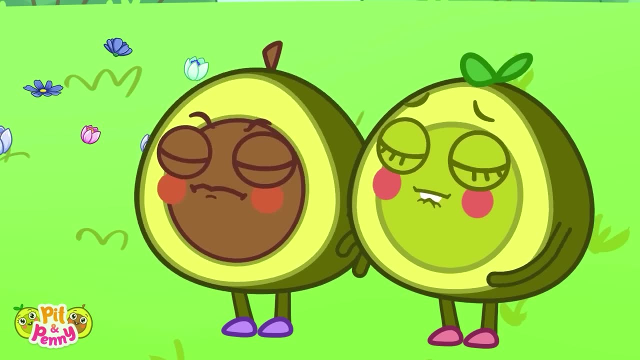 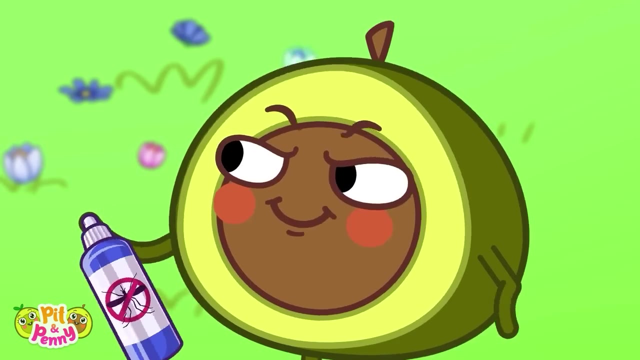 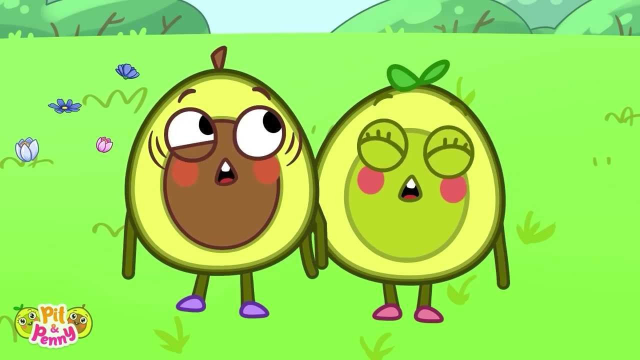 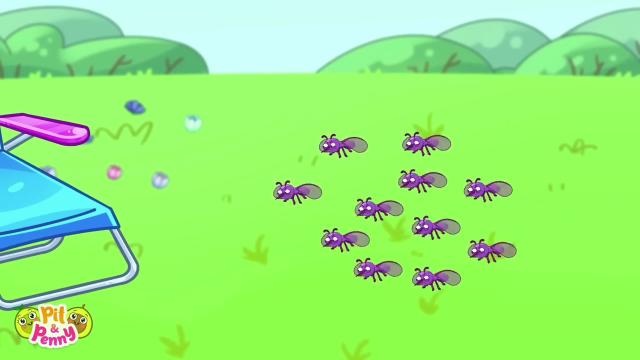 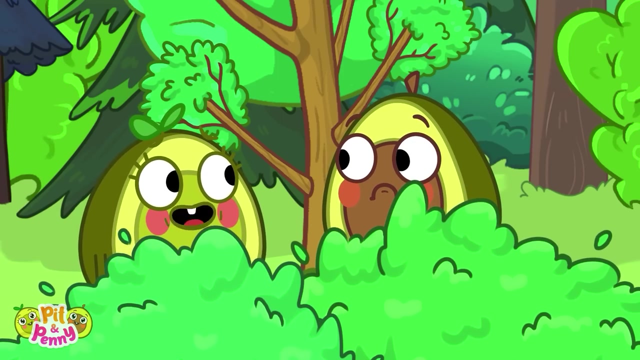 Pit will help. Oh, Oh, Oh. What should Pit do? He'll use bug spray, of course. Thank you, Pit. More mosquitoes, Quick Hide in those bushes, Pit. What do we do now? What can Pit do with a branch? 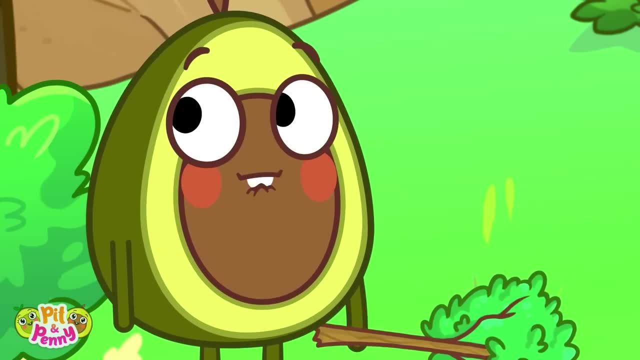 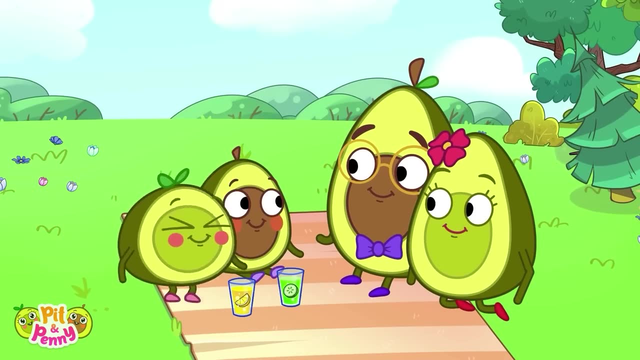 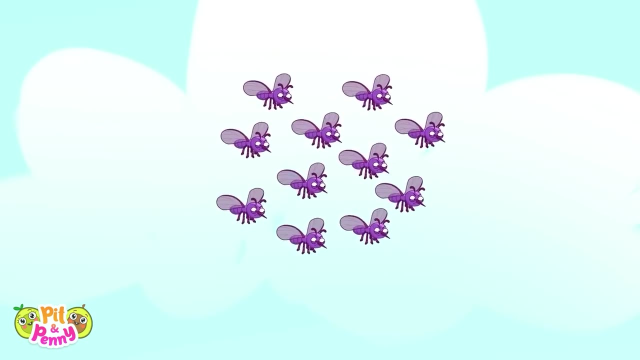 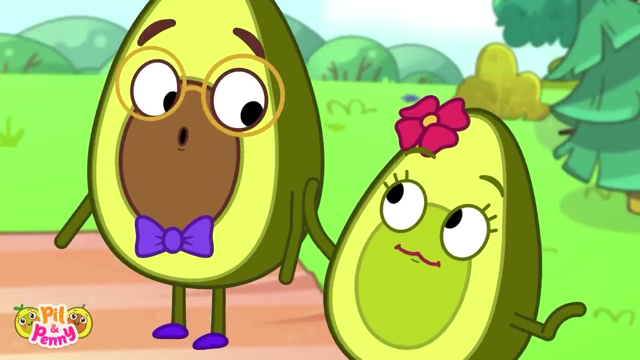 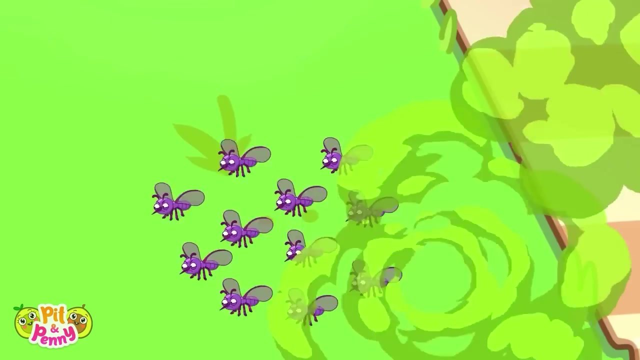 Ah, the branch is a fly swatter. What a good idea. Pit Time for a refreshing drink? Not again. It's good we have insect repellents. It's Baby, She'll use bug spray to shoo those mosquitoes away. 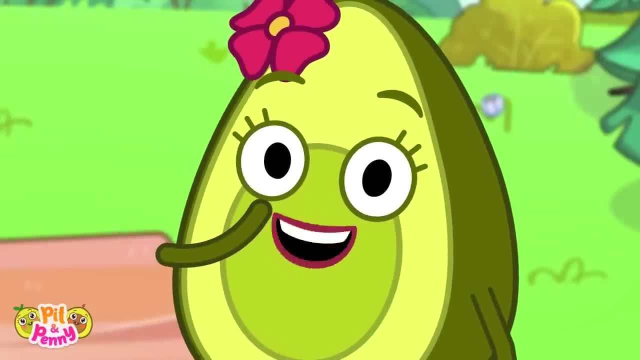 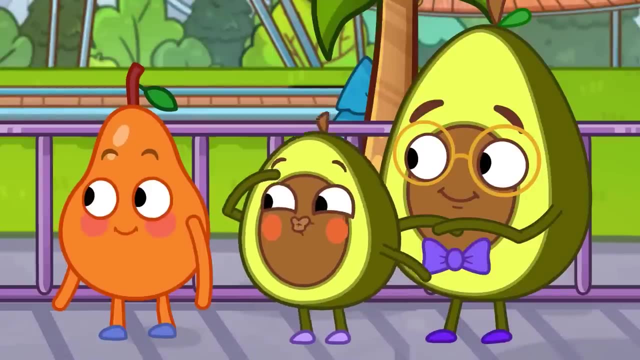 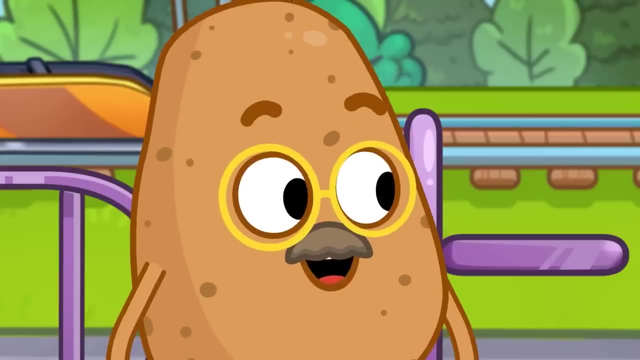 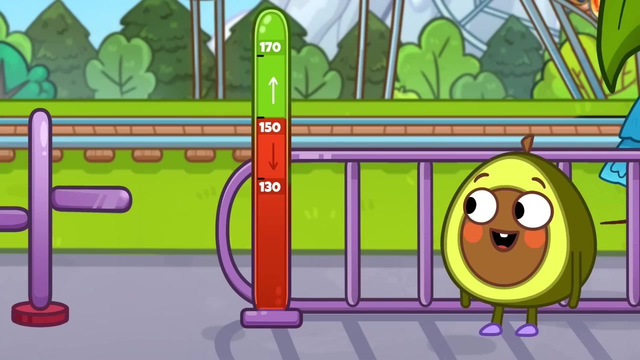 That's better. Don't forget to protect yourself from mosquitoes and their bites. Now back to the picnic. Pit is waiting in line for the roller coaster. Is Perry tall enough to ride? Yes, he is. Okay, it's Pit's turn. 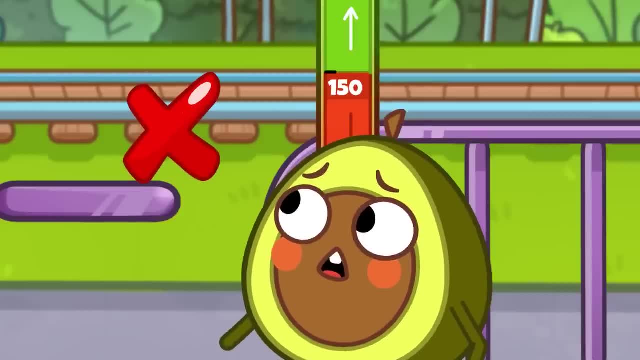 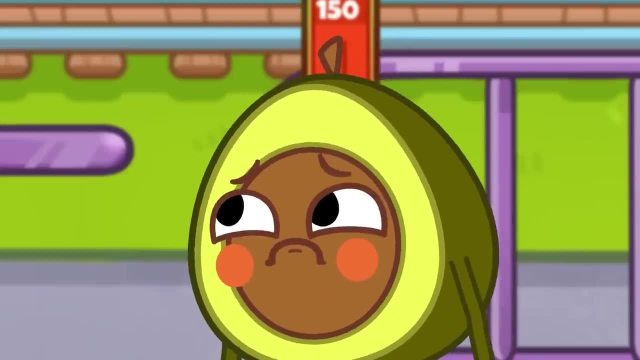 Ah, Pit is too little for this ride. No, Pit is too little for this ride. Too short, Poor Pit. What would make Pit feel better? Ooh, Maybe some ice cream. I know how to cheer you up, Pit. 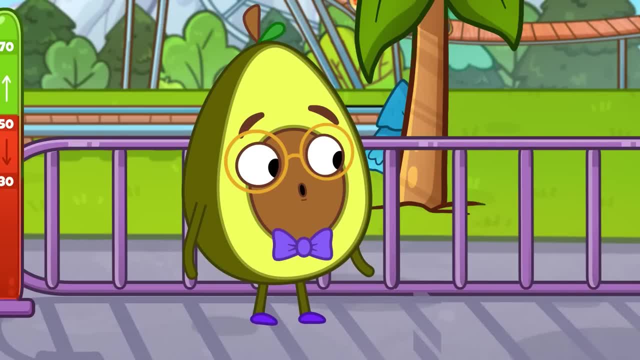 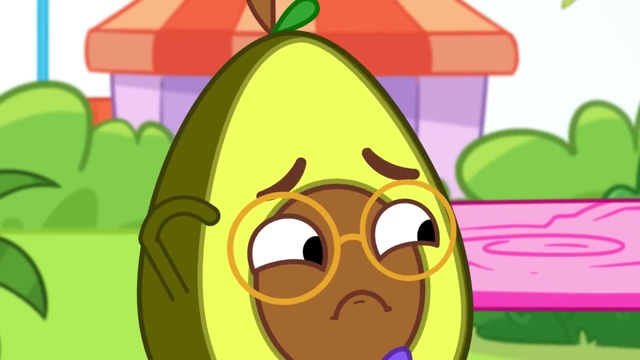 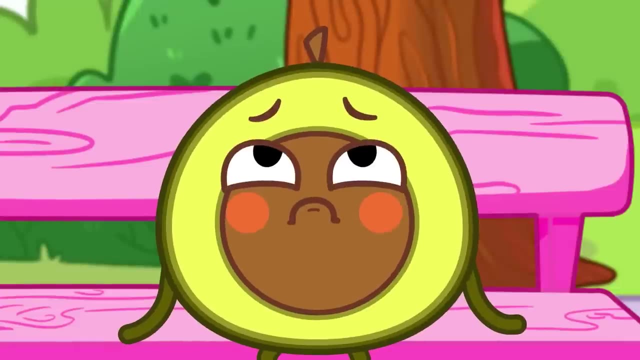 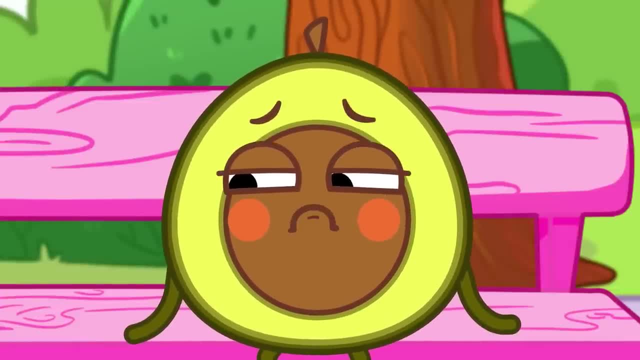 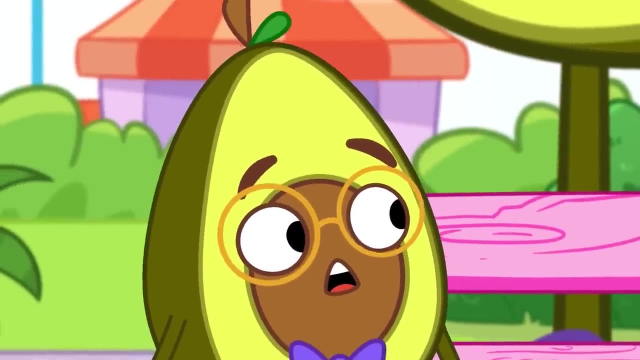 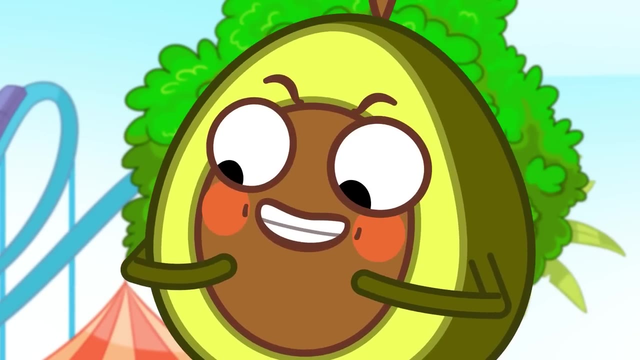 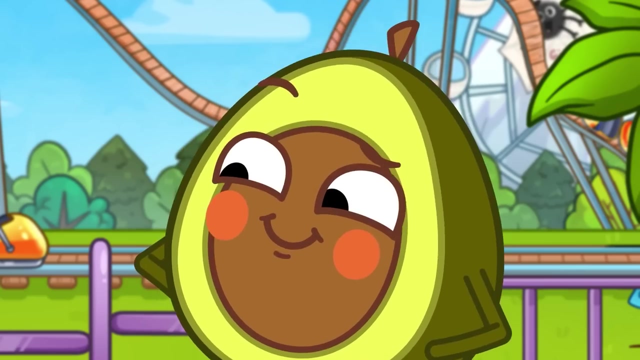 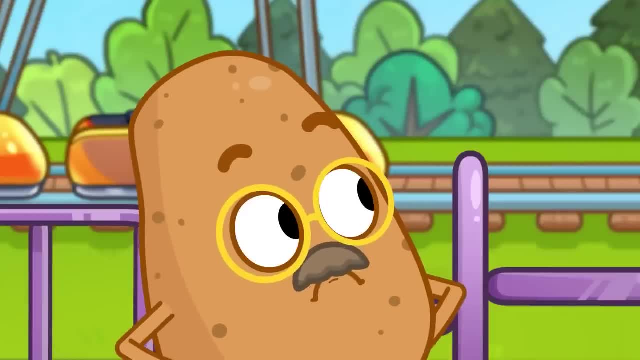 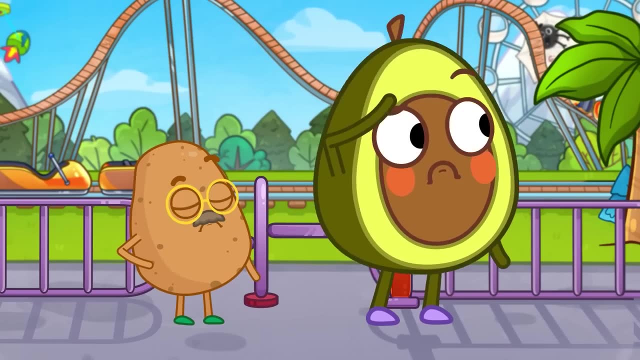 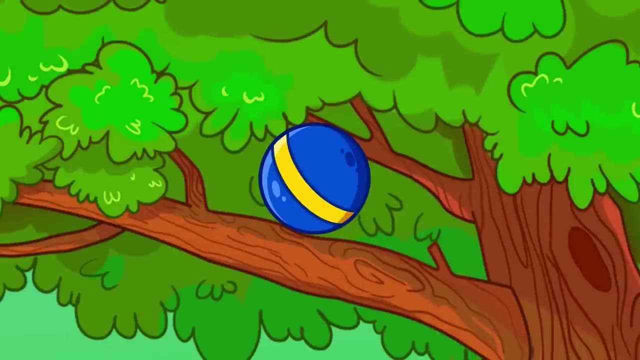 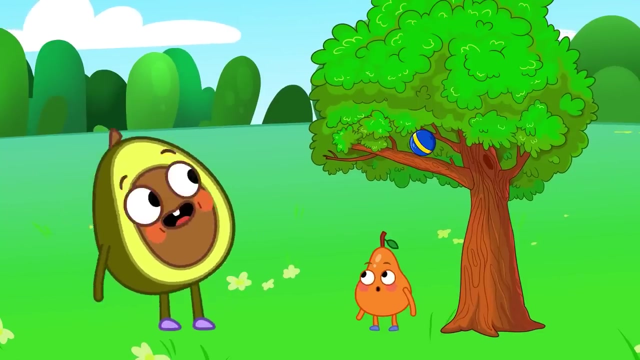 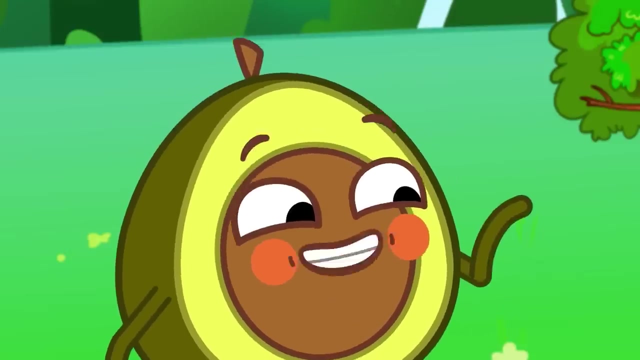 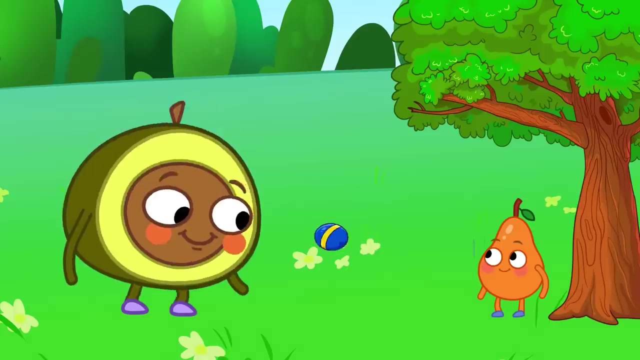 But why not? Mm-mm, Too tall, No entry. What is it? Pit Harry's ball is stuck in a tree. Maybe Pit can get it out. He did it. Let's play together. Pit is too strong now. 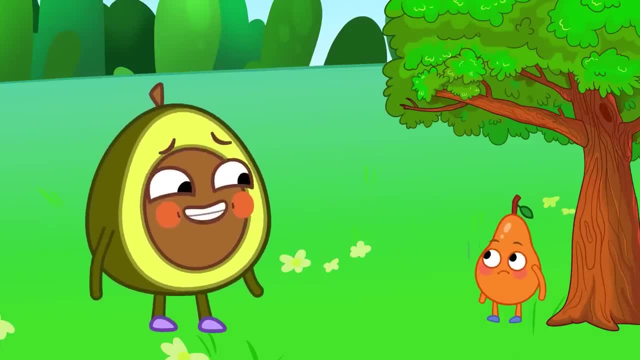 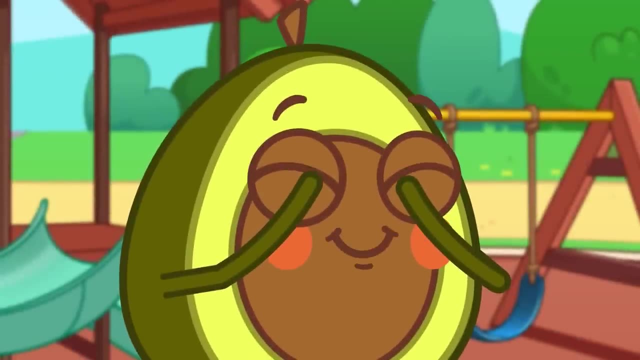 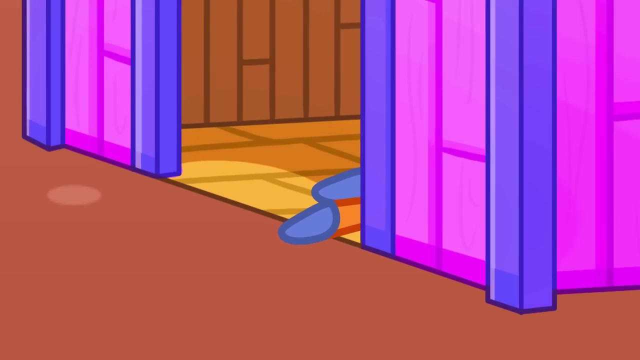 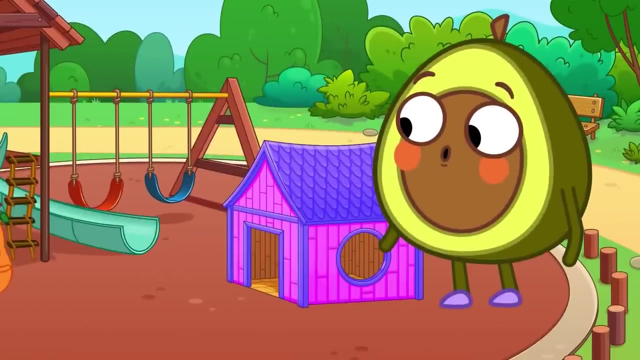 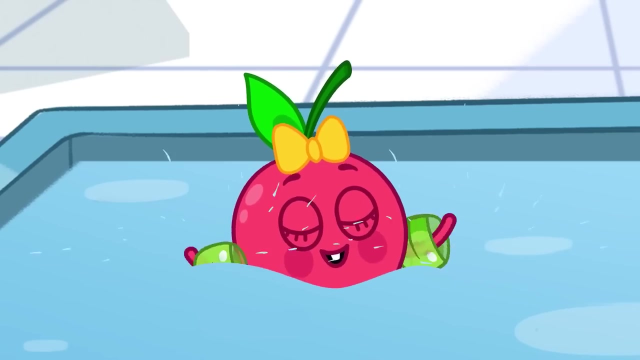 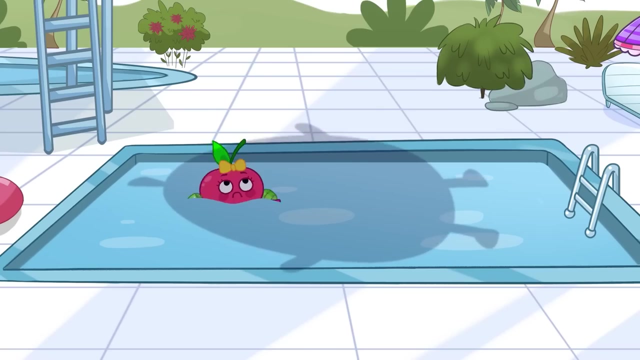 Bye-bye ball. Can we play hide-and-seek Three, two, one. Where is Perry hiding? Pit found Perry, But Perry's afraid to play with a giant Cherry is swimming. Pit wants to swim too. Oh no, The water's all gone. 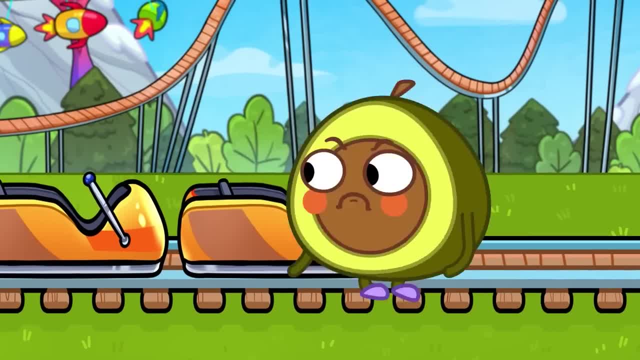 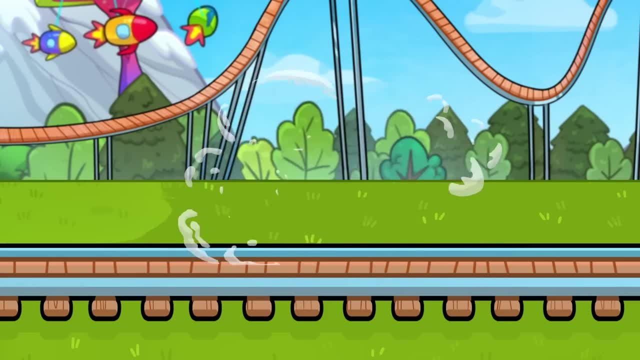 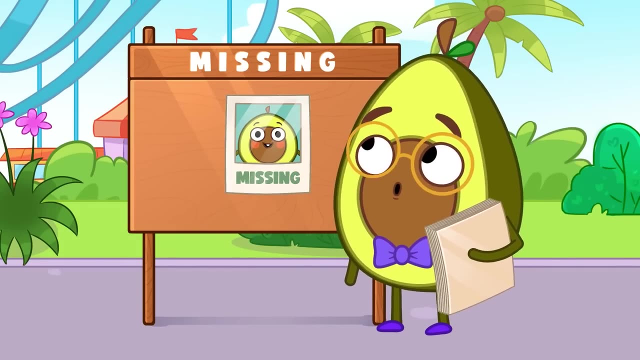 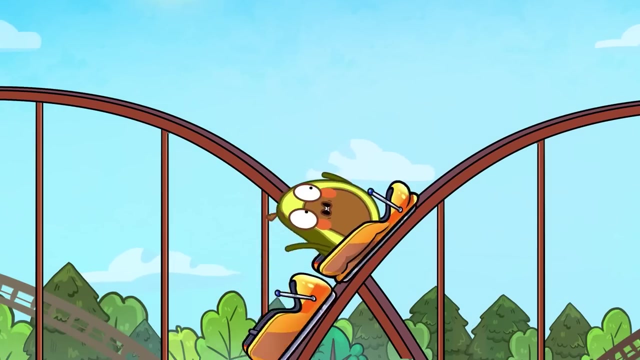 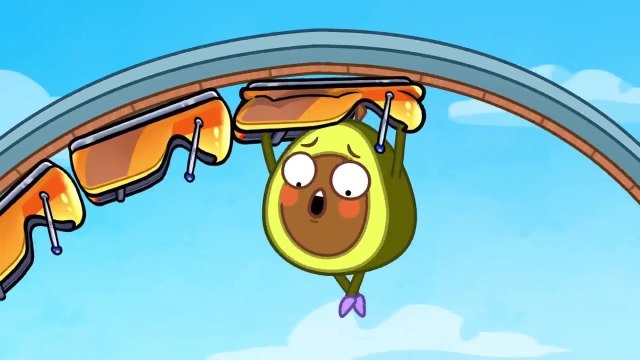 No, Pit, You're too big. He isn't following the rules. Daddy is looking for Pit Pit. Pit is stuck. Pit is stuck. Pit is hoping it's about to fall. Well done, face. Try to stay at my feet. 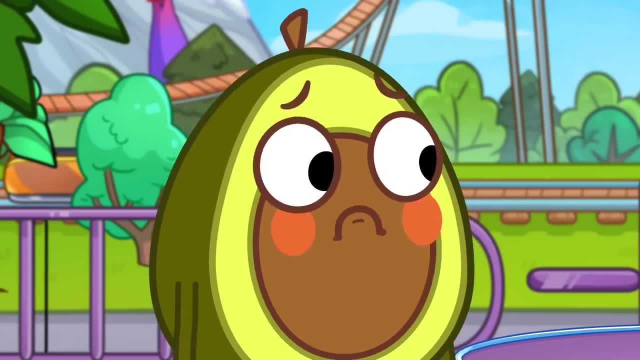 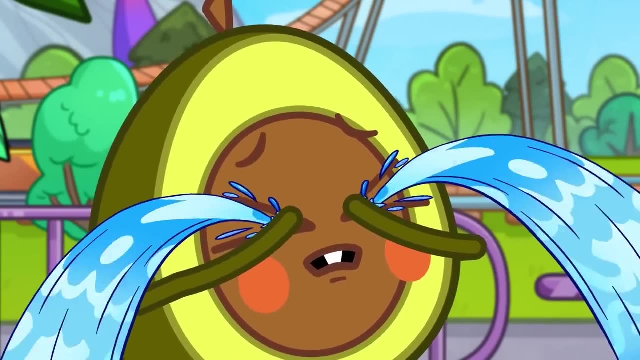 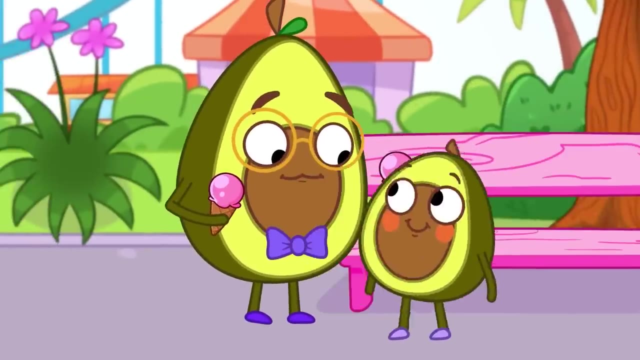 I'm sorry, vest, Watch your back. baby Tagt, it's so wide Man, isn't it too hot in here? It's right below the tree. Let's see if it can drive home, Rhett, What? 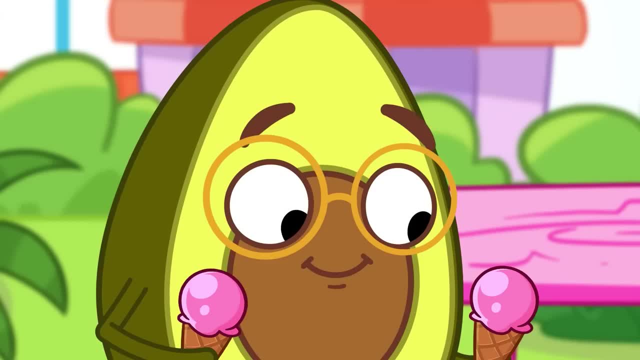 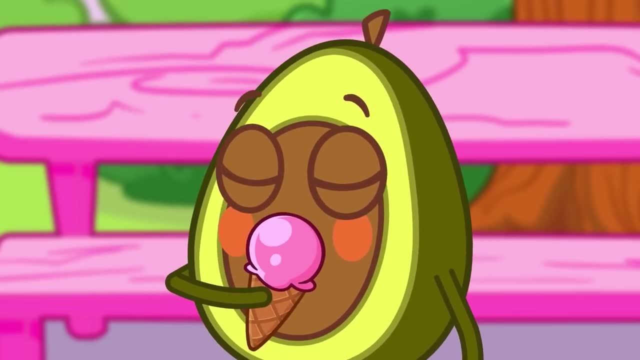 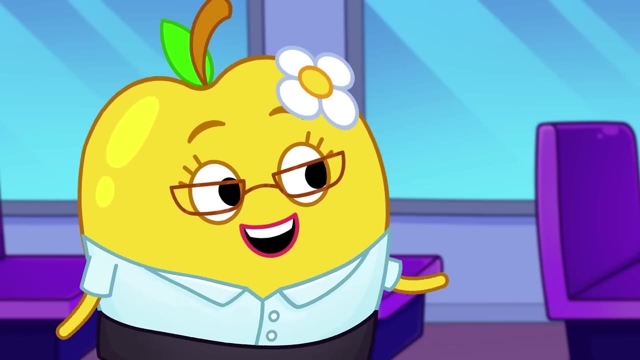 Oh, I won the race. This is crazy rail. One day you will be as big as me, But you're the perfect size for ice cream. Here comes the school bus. Slow down, Pit and Penny knocked over Miss Apple. 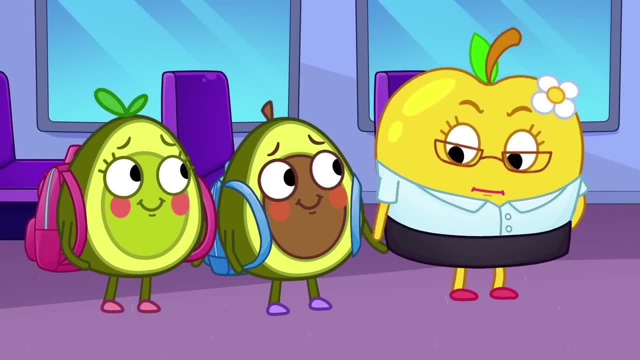 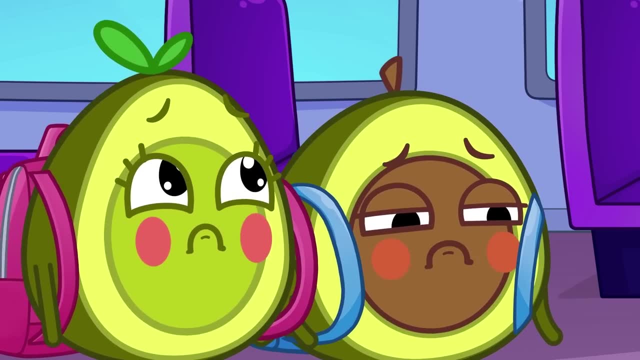 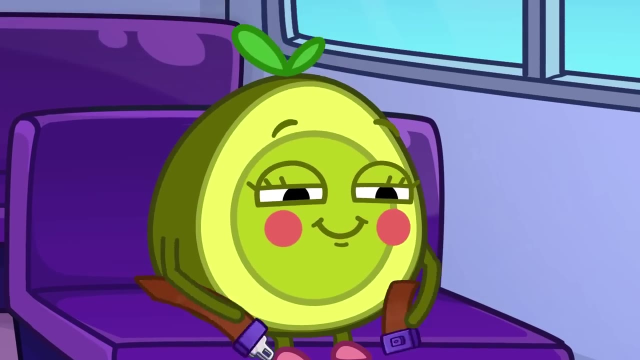 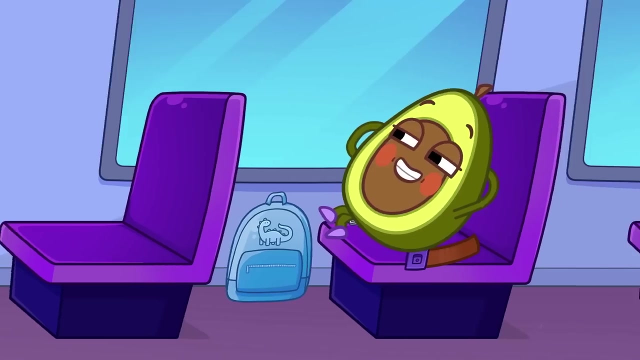 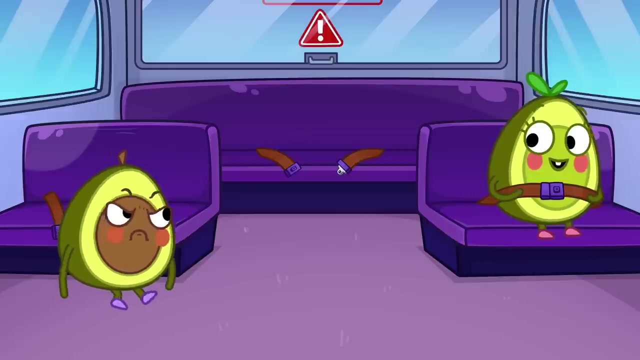 Help Miss Apple up, please. You can't run on the bus. I'm sorry, Find your seats. Penny buckles up. Pit doesn't like wearing seatbelts. See what happens, Pit, Pit. you must obey the signs. 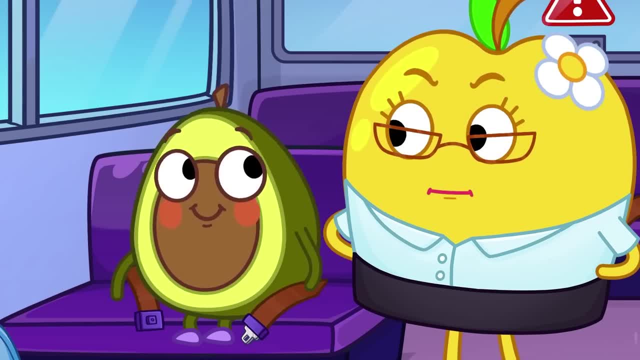 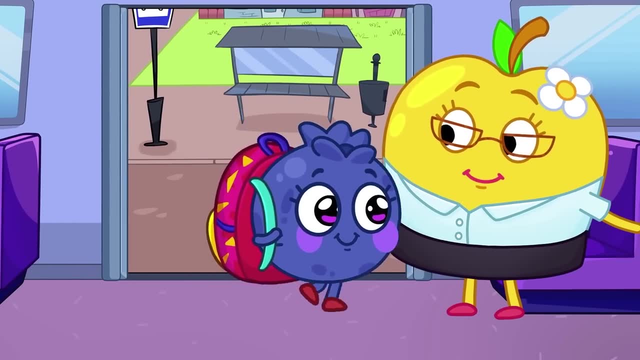 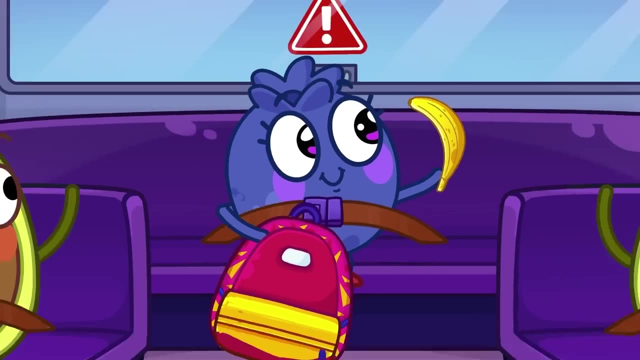 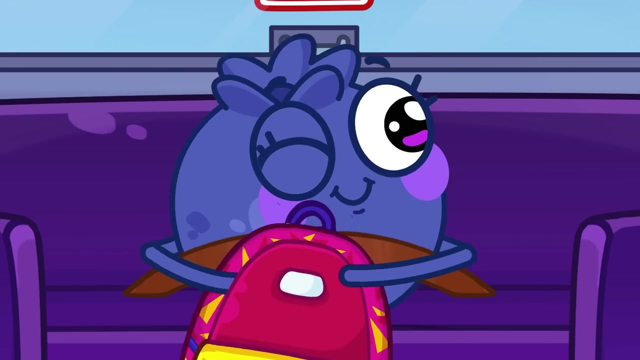 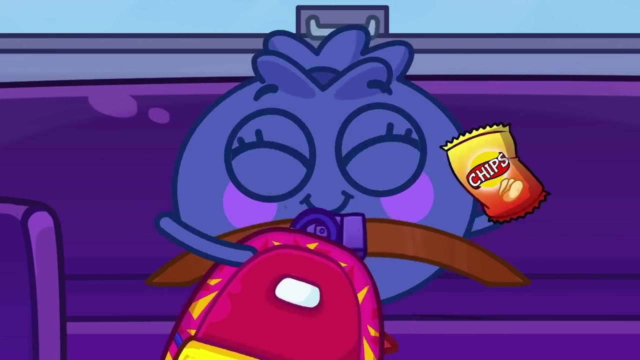 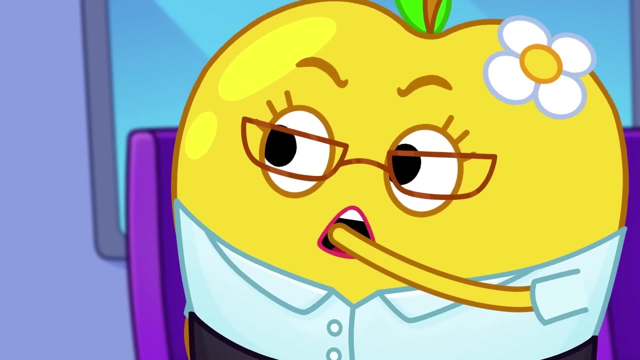 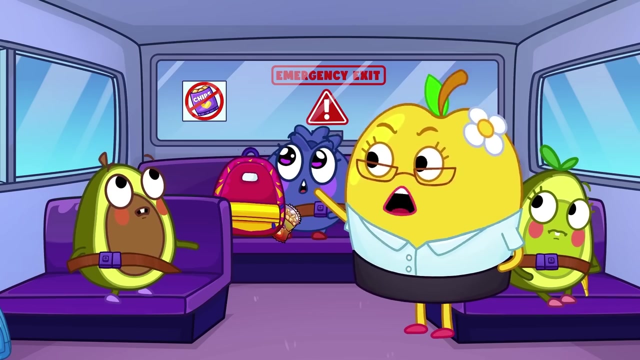 You need to fasten your seatbelt On the bus. Blueberry brought snacks: A banana for Penny, A banana for Pit And chips for herself, But you shouldn't eat on the bus. What does the sign say? You can't eat on the bus, especially unhealthy foods. 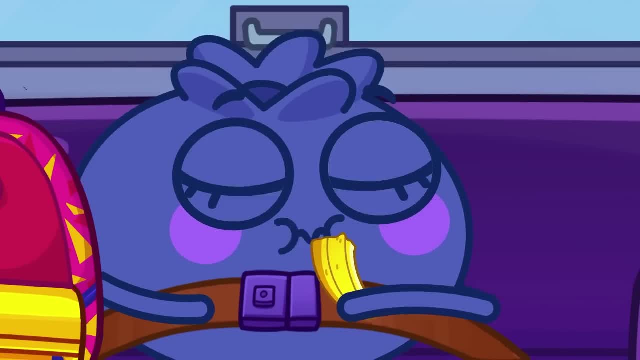 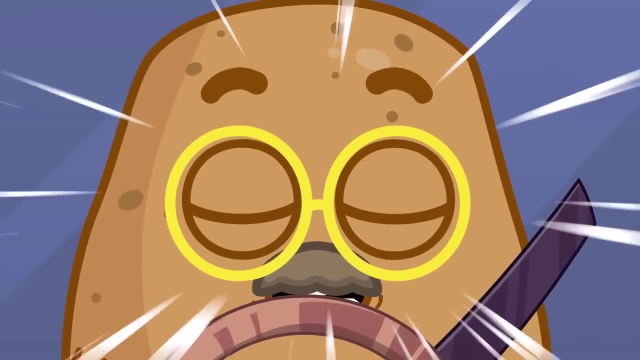 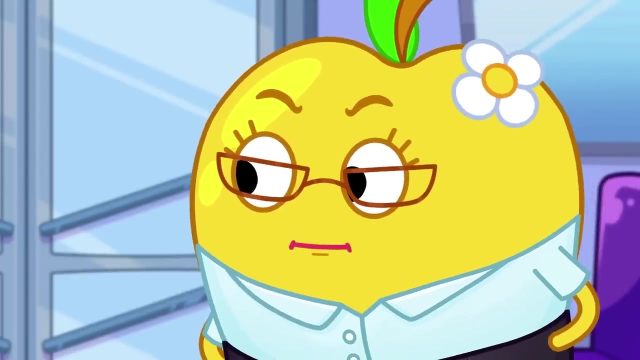 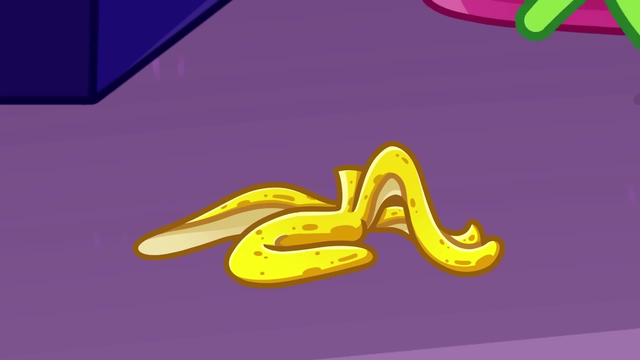 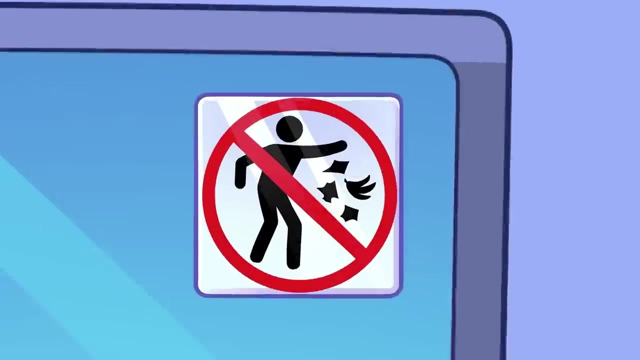 Penny, it's nice to share, but you should put those snacks away. It's Lime and he's late for the bus. Don't miss the bus. Lime, watch out. This is why you can't eat on the bus. Your litter can hurt other people. 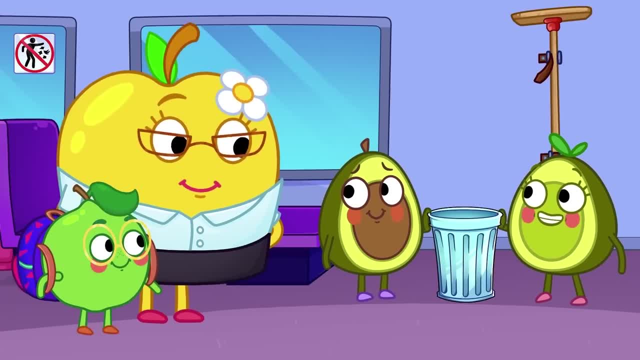 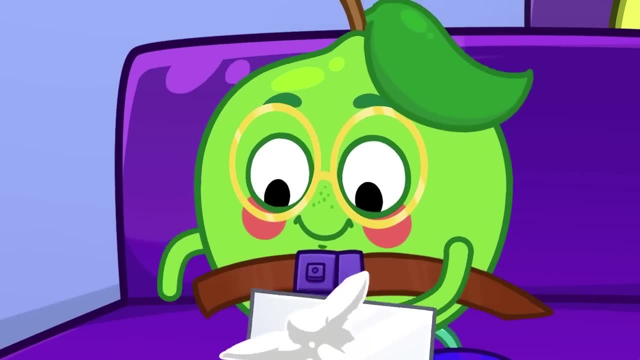 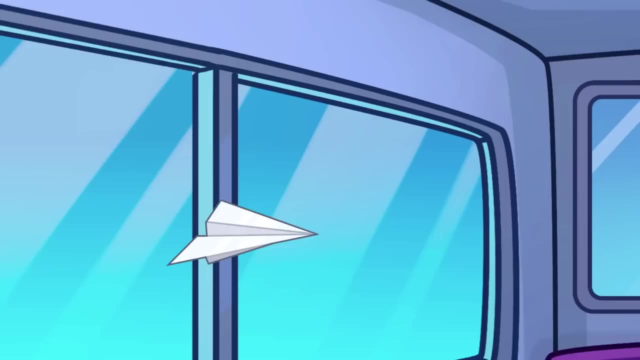 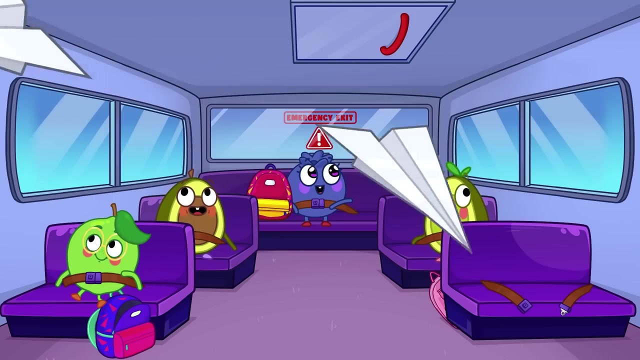 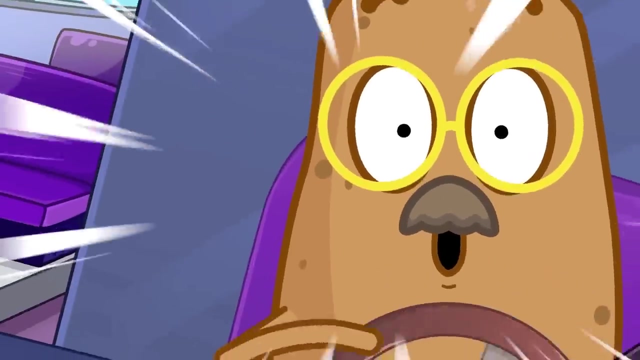 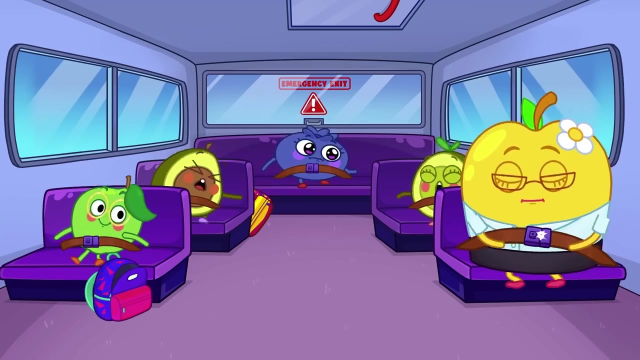 Your banana peels belong in the trash. Lime is bored. He made a paper airplane. Now all the kids want to make one, But don't throw them on the bus. They covered the driver's window. Hold on kids. Phew, Everyone is safe. 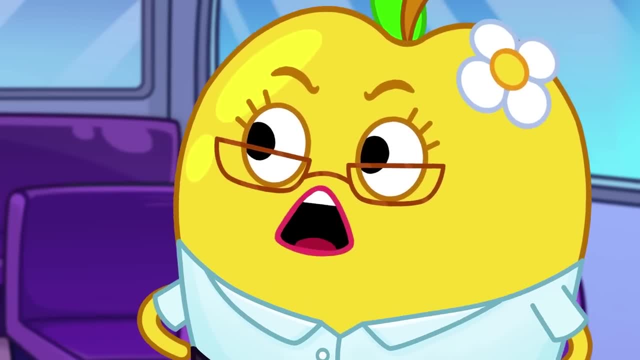 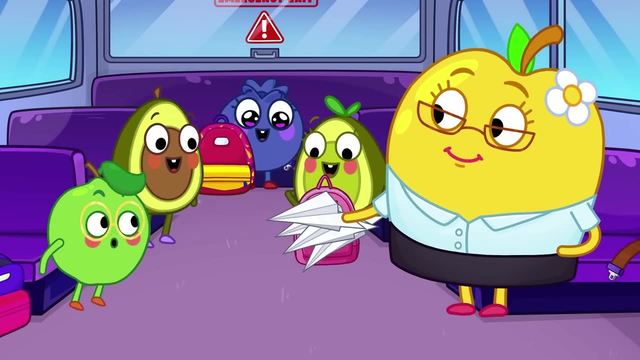 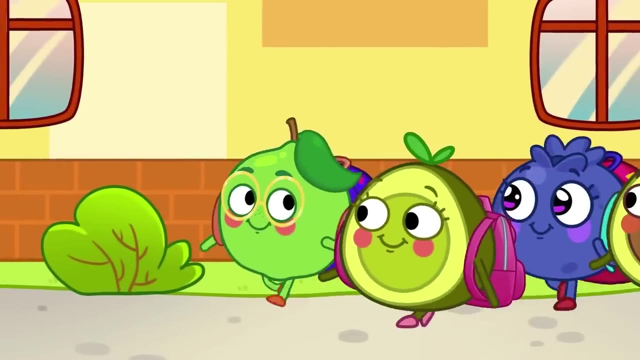 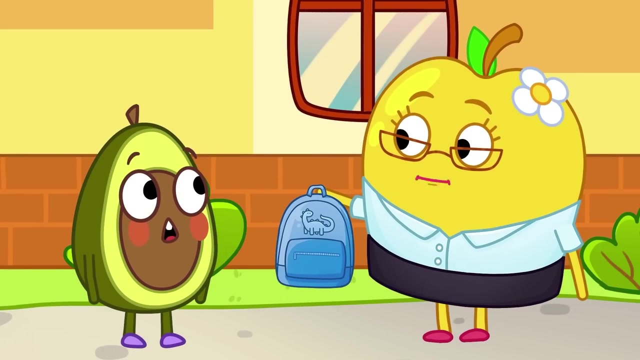 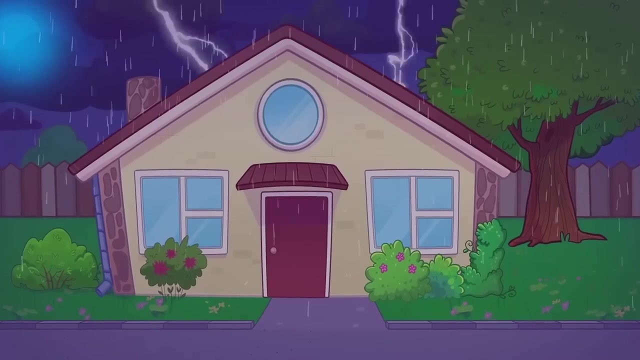 This is very dangerous to play games on the bus. I'm sorry Time for school, But Pit forgot his bag. Don't forget your things on the bus. Now you can have fun at school. Bye, kids, It's a stormy night. 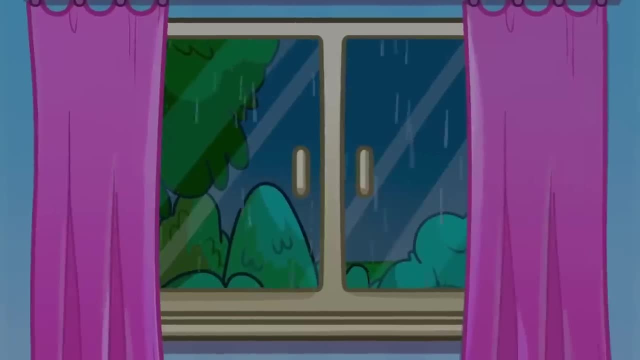 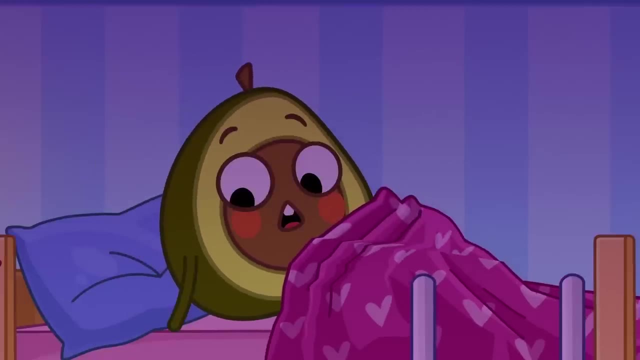 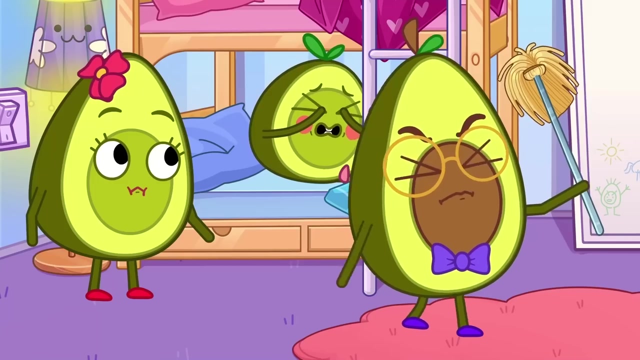 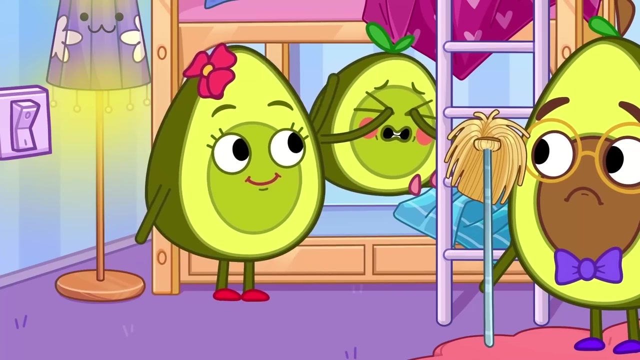 And Pit and Penny are tucked up in bed. A storm has woken them up. A storm has woken them up. Penny is scared. Don't worry. Mommy and Daddy are here, They'll make sure everything is okay. Mommy tells Penny that there's nothing to worry about. 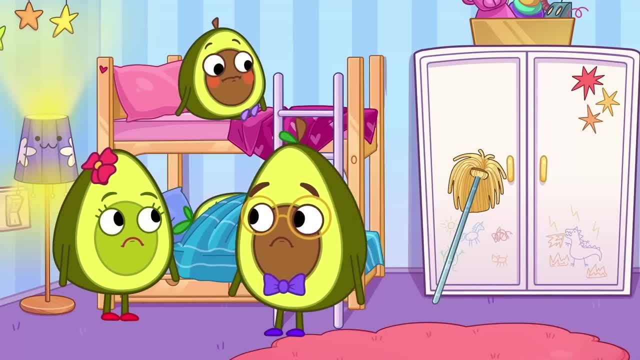 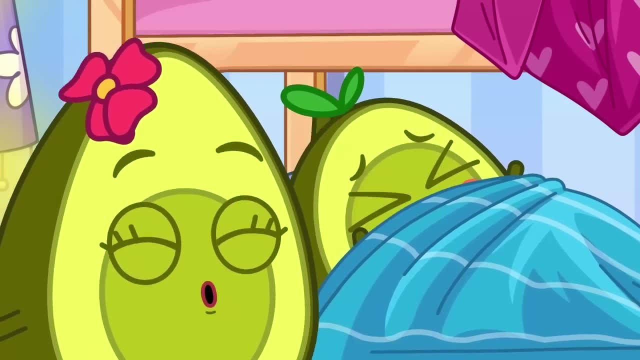 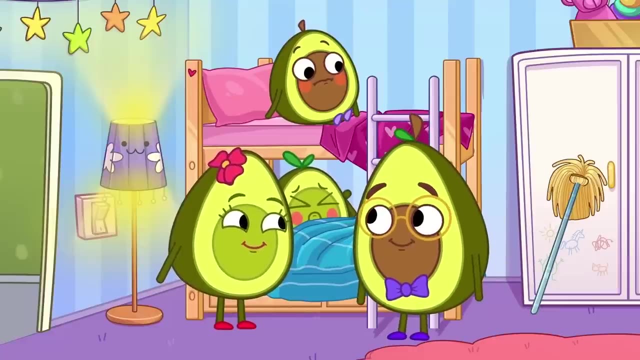 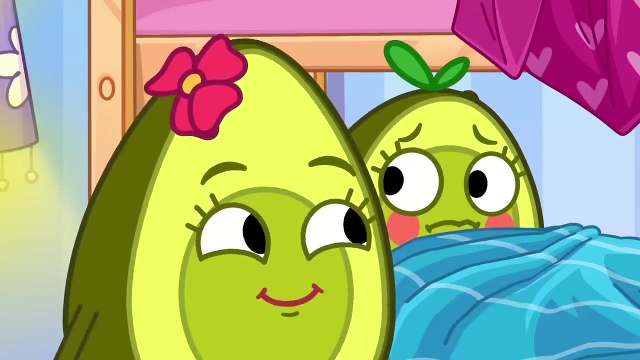 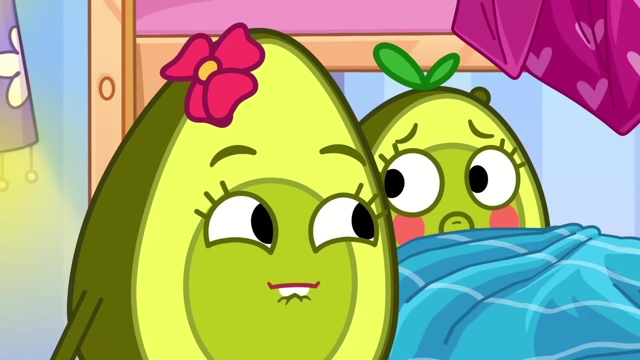 Oh no, There's more thunder and lightning. Don't be afraid of the storm, You're safe here. Let's count together: One, two, three… With every number, the thunder gets farther. Repeat after me: One, two, three, four, five…. 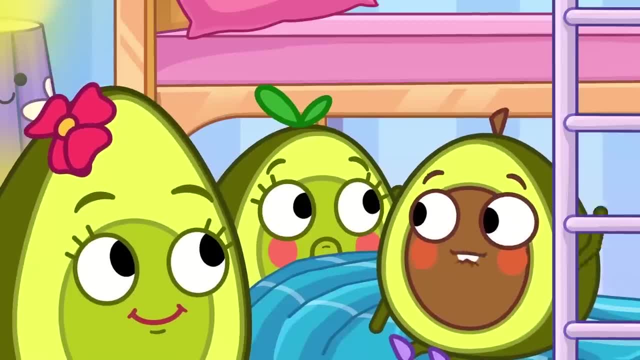 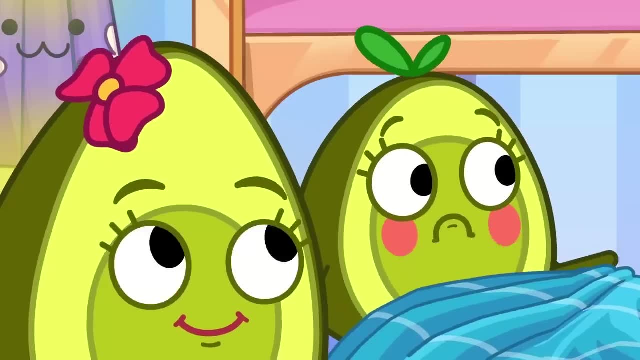 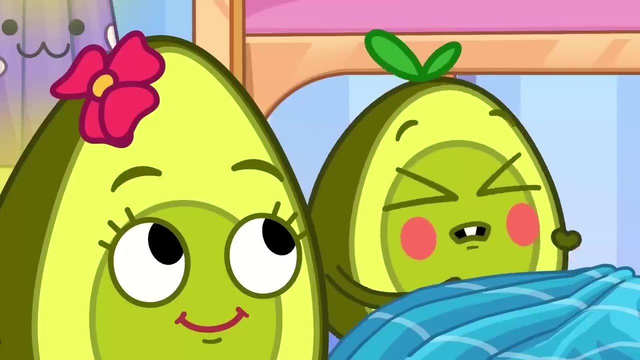 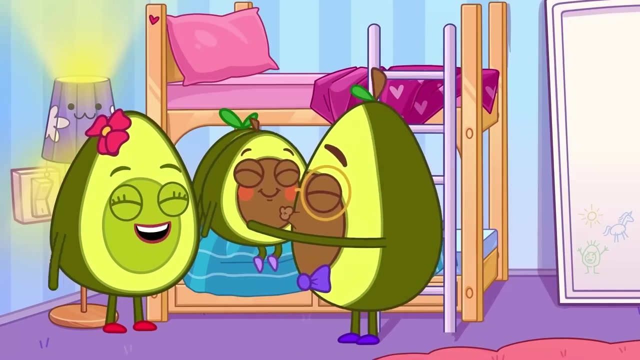 Oh no, Oh no, Look, The thunder goes far, far away. Pit's right: One, two, three, four, five, six, seven… It worked, Mm-hmm Aww. Now everyone can go to sleep. 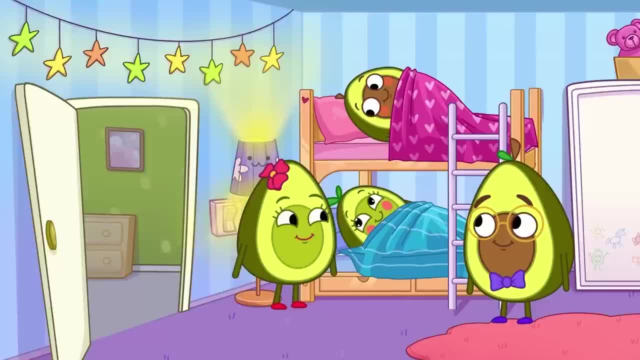 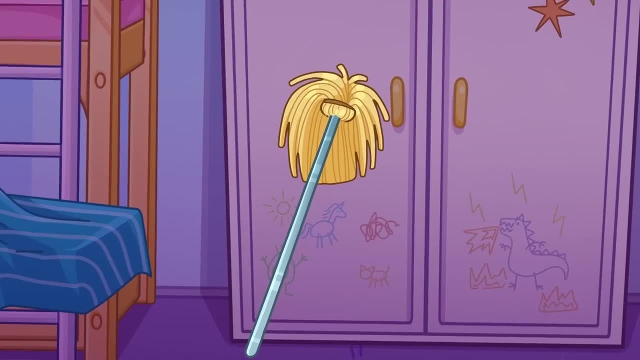 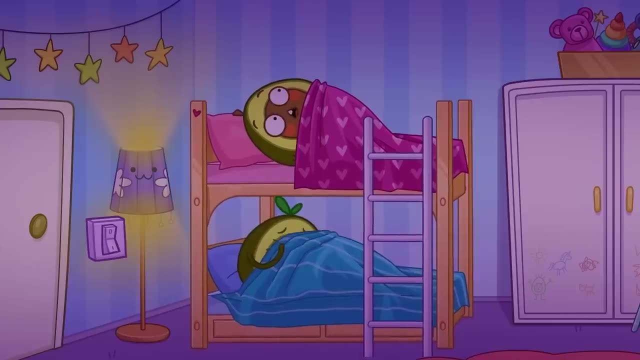 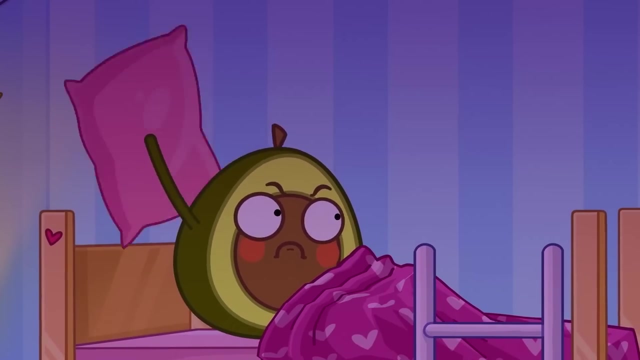 Aww, It's time for a little nap. Time for sweet dreams. Time for sweet dreams. Time for sweet dreams. Penny has seen a monster. Penny is frightened again. Pit knows how to fix things. Nice shot Pit, Nice shot Pit. 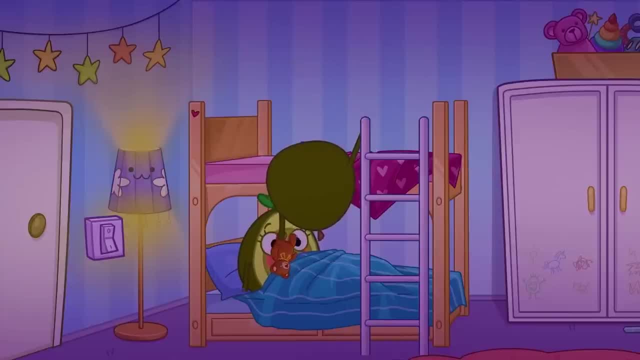 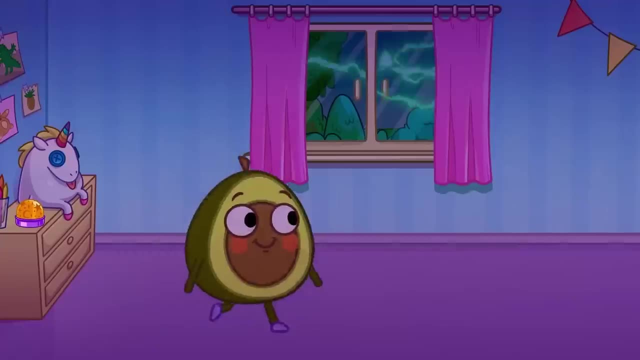 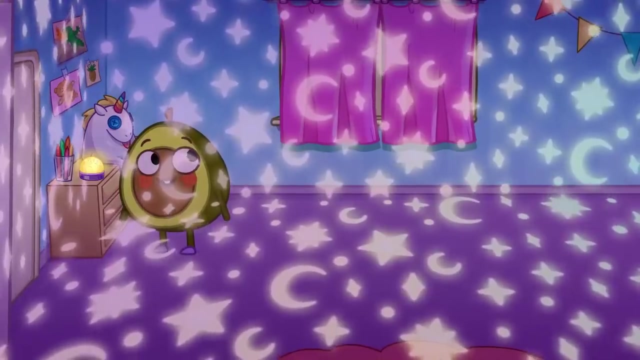 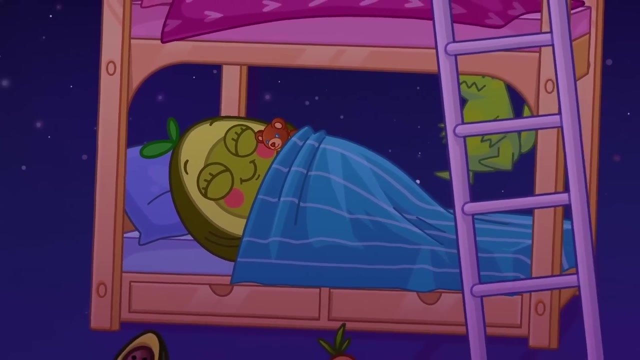 Goodbye, Goodbye, Goodbye. Aww, Pit is sharing his teddy bear. That's very kind, Pit. Now we can't see the storm. Look at all the stars. Sleep tight, Penny. Penny is dreaming. This looks like a nice dream. 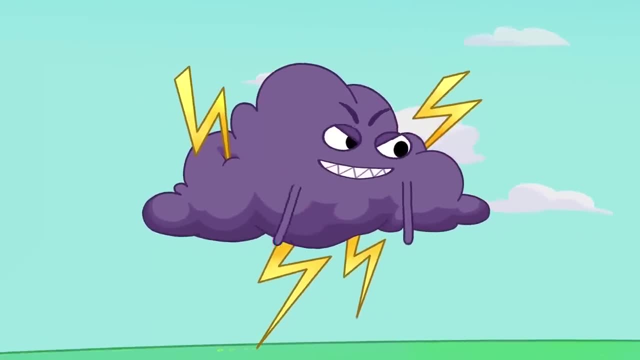 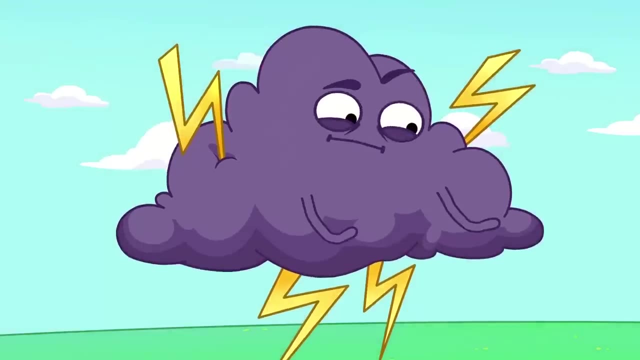 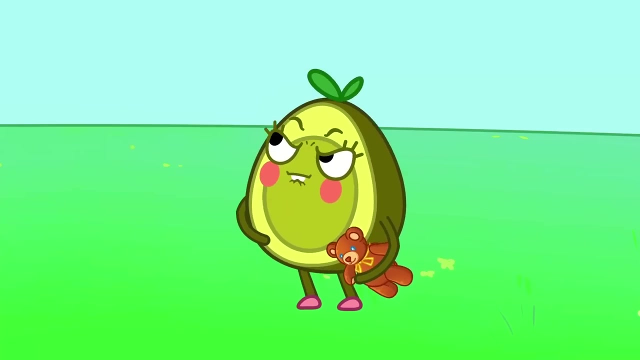 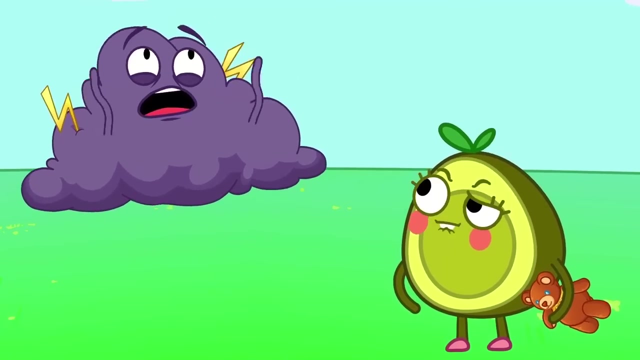 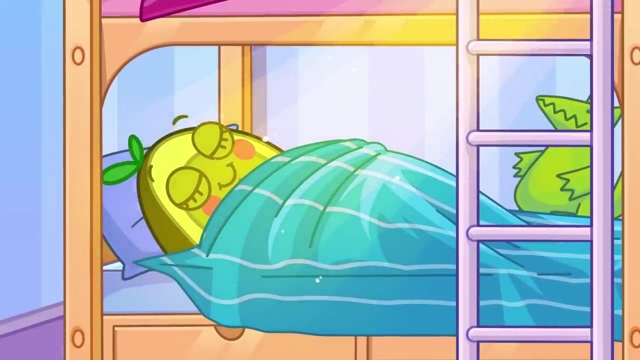 Hey, There's a storm cloud in Penny's dream. One, two, three. One two, three, four, five. Penny isn't scared. One, two, three, four, five, six, seven. It's time to wake up, Penny. 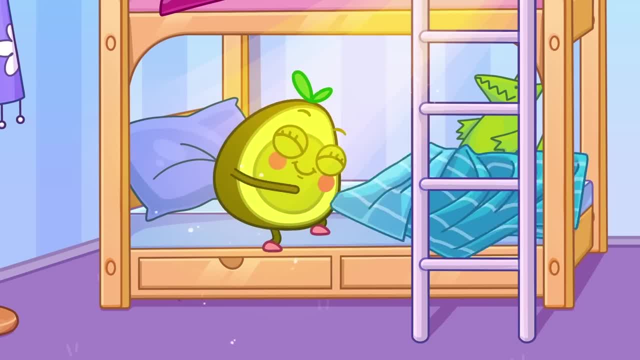 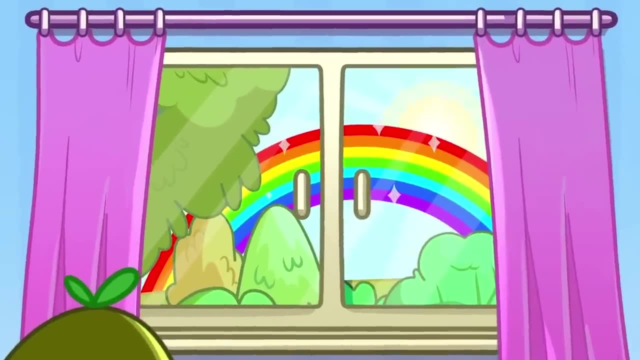 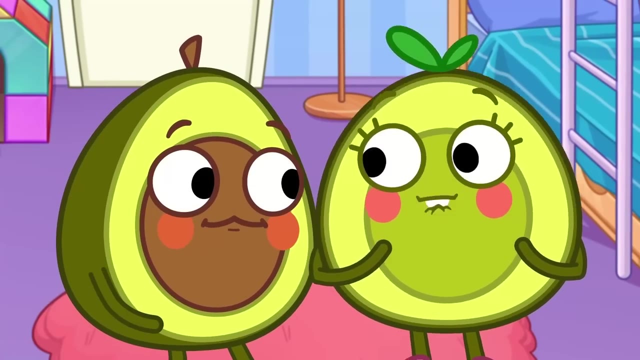 It's a bright, sunny day. There's no need to be scared. Penny sees a beautiful rainbow. There's always a rainbow after the rain. It was totally worth waiting for. It really was Penny Shh. Oh no, Oh no. 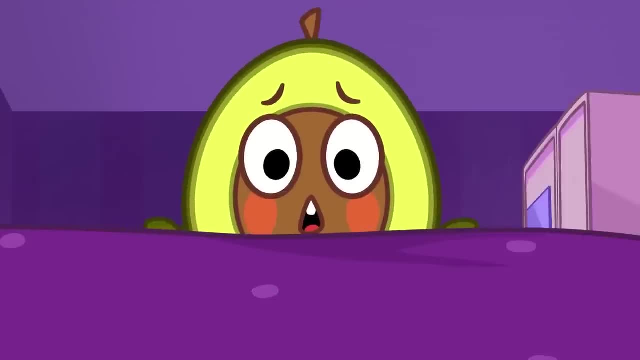 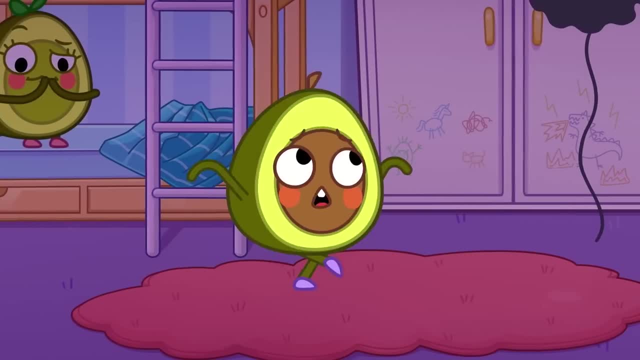 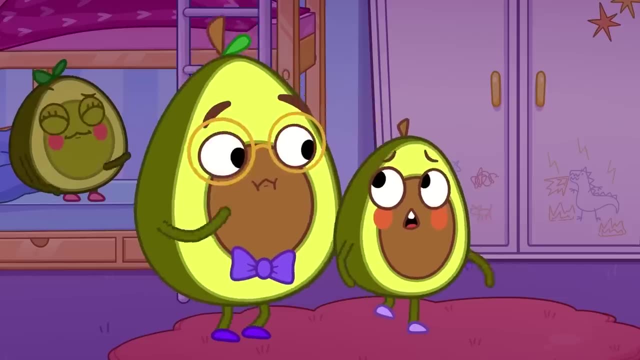 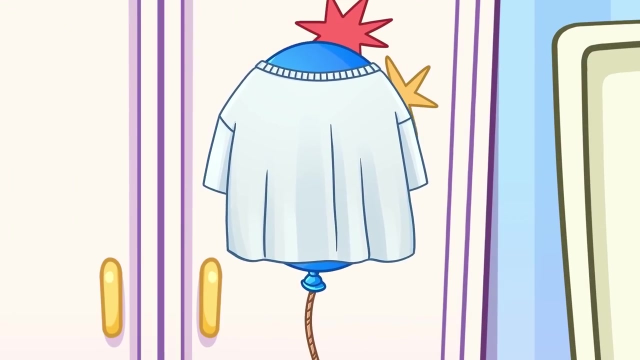 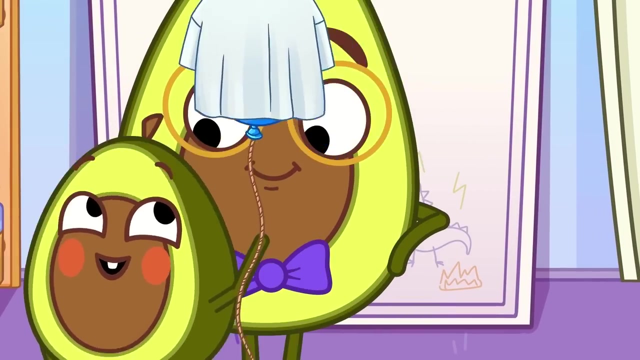 There's a ghost flying over my bed. There it is. Mm-hmm, Don't worry, Ghosts don't exist, It's just a balloon in a t-shirt. I had no doubt. I had no doubt. Okay, everyone back to bed. 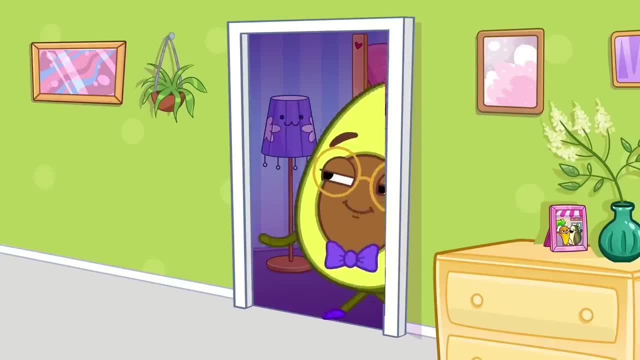 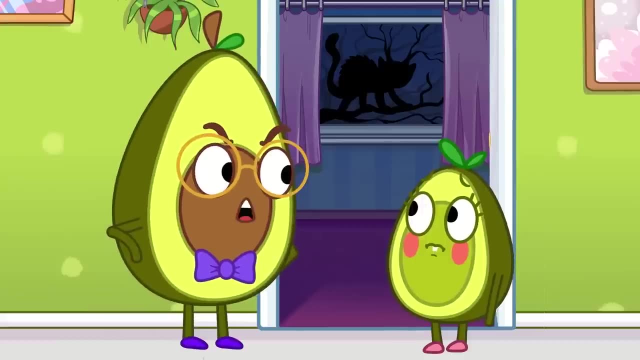 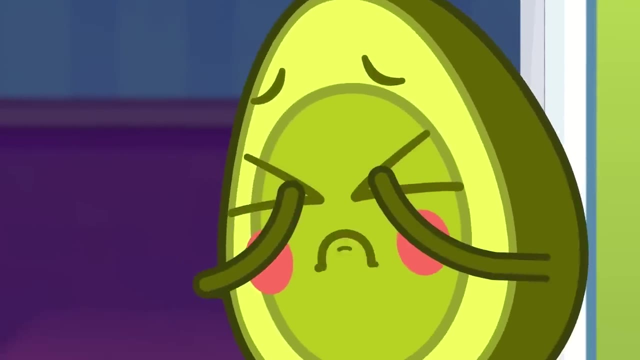 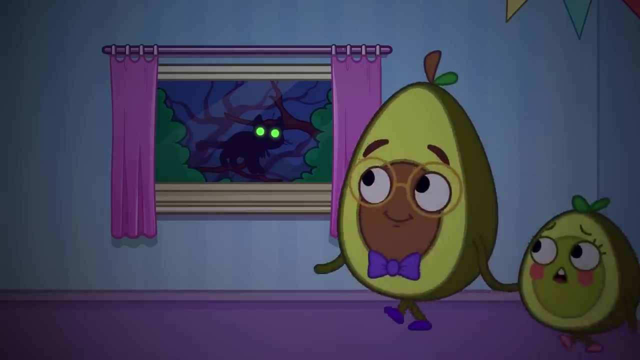 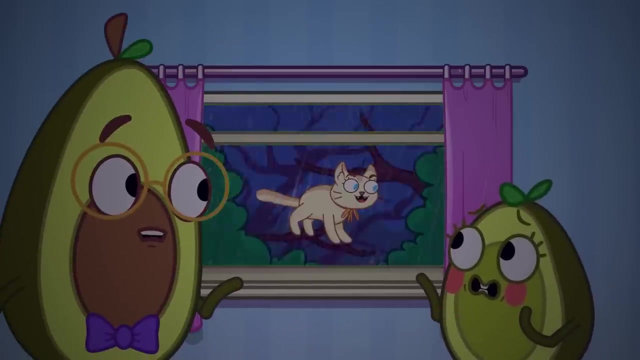 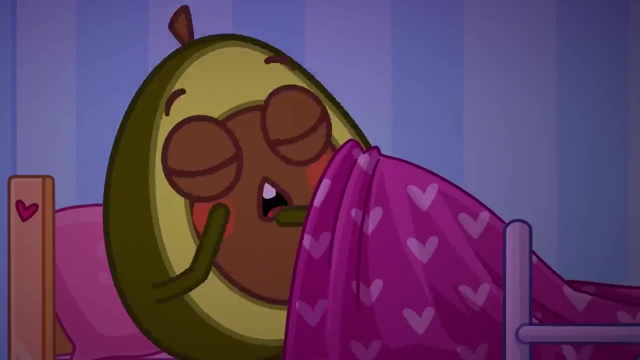 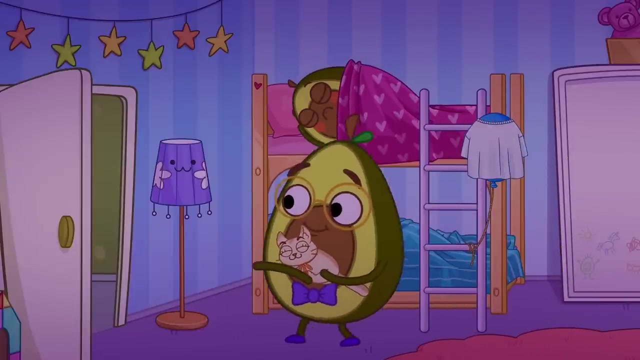 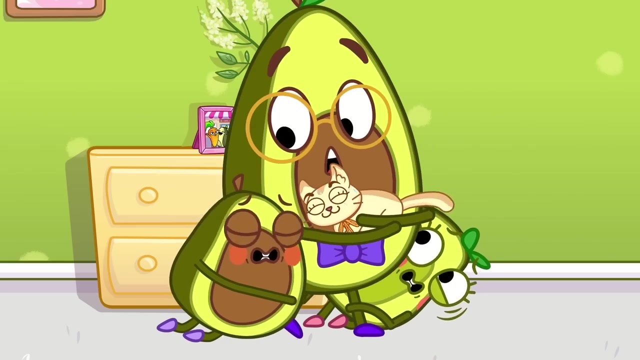 Don't be scared, Daddy, It's just Penny. Penny, why aren't you asleep? There is a monster watching me. Let's see what it really is. It's not a monster, It's just a cat, And I wasn't scared at all. Now, Pit and Penny are both scared. 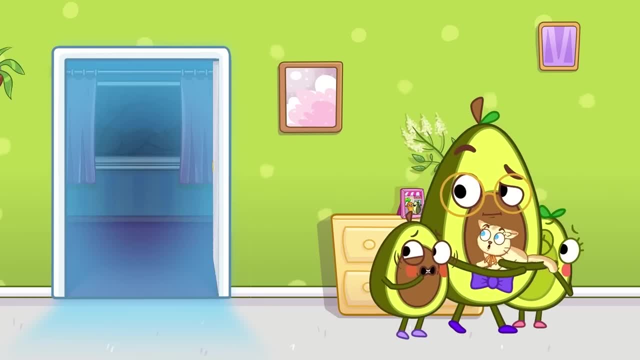 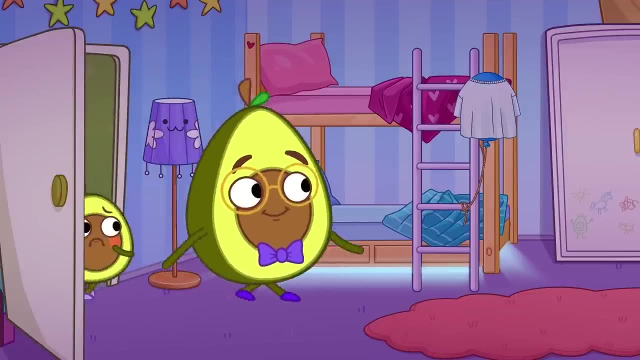 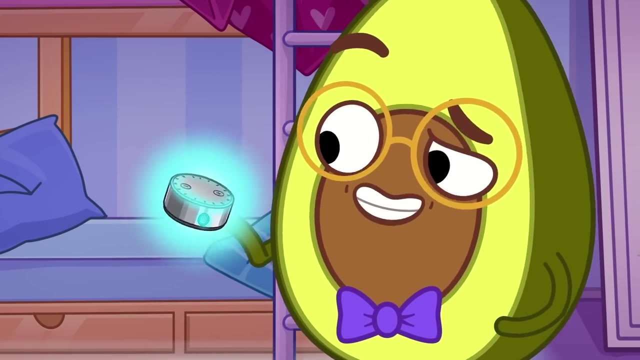 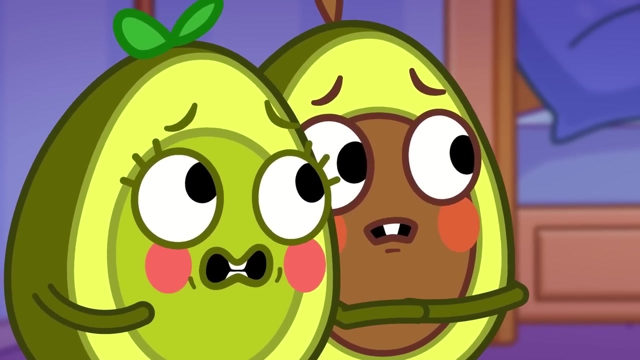 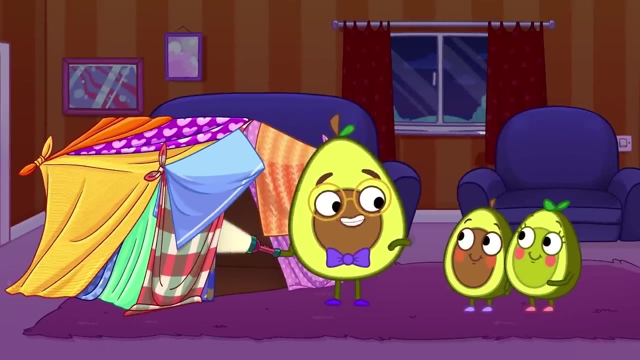 There's a strange light in their room. Daddy will check it out. It's under the bed, Daddy. Aha, It's just a toy, Dad. we're not sleeping here. Daddy has an idea. You won't be disturbed here. Yay, It's a blanket fort. 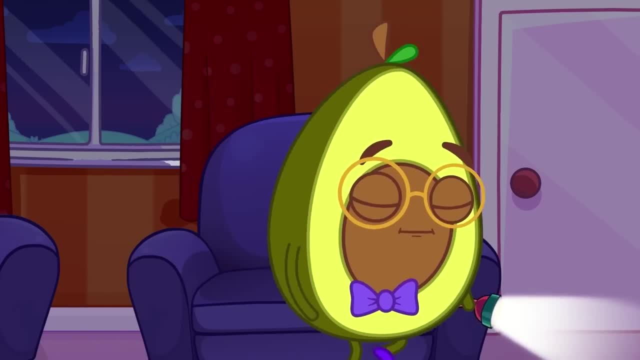 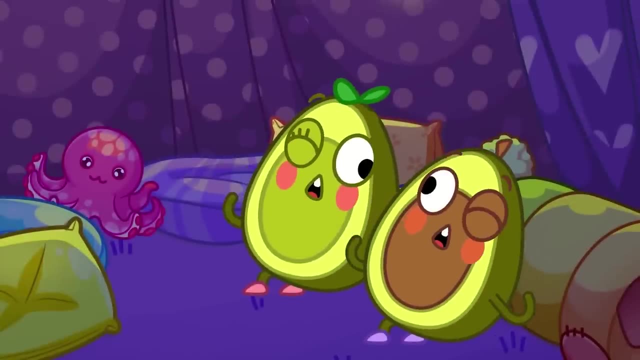 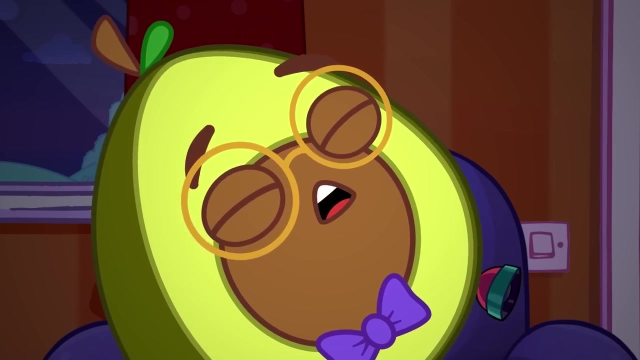 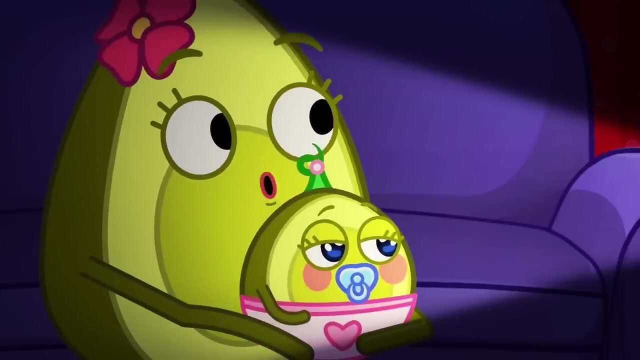 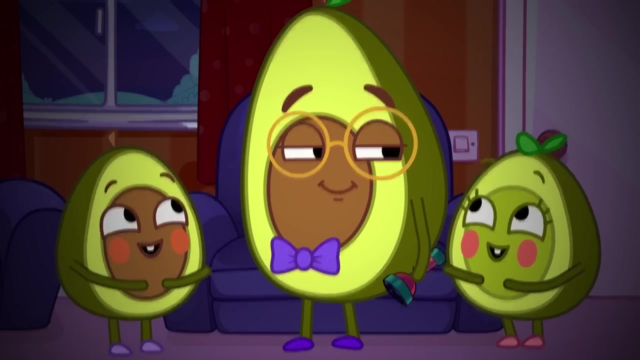 How cozy. Maybe now Daddy can get some sleep. Oh, some sleep And scary shadows. DADDY, HELP US, THERE IS A MONSTER. Sleeping in the living room isn't the best way out. Better make a night light Now everyone can sleep. 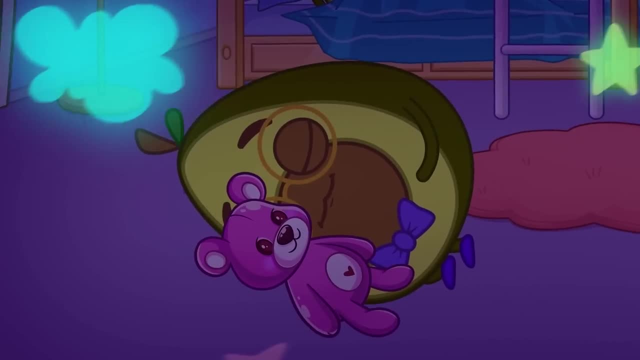 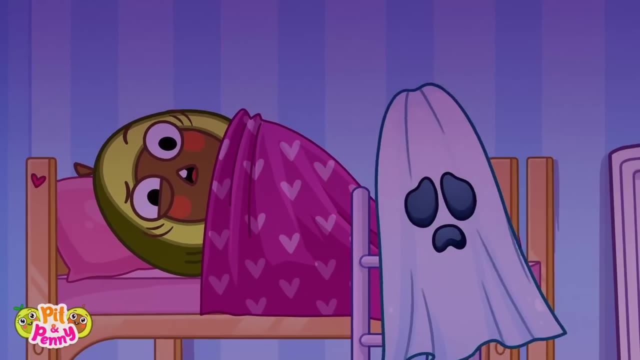 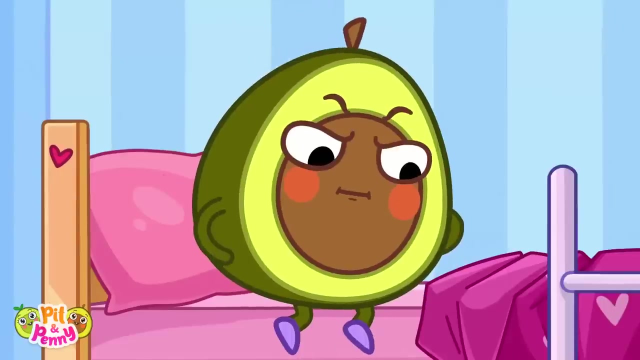 Even Daddy. Ok, let me help you. Thanks, Daddy, How do you like it? I think this one is more fun than the others. Your dad and I agree. I'm proud of you, Polly, swimming with your daddy. What's that Pit? It's just Penny playing a prank. 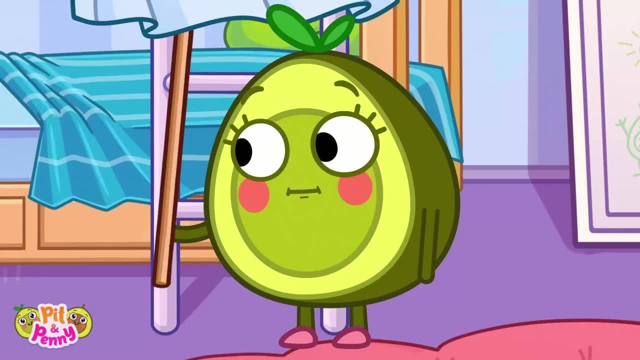 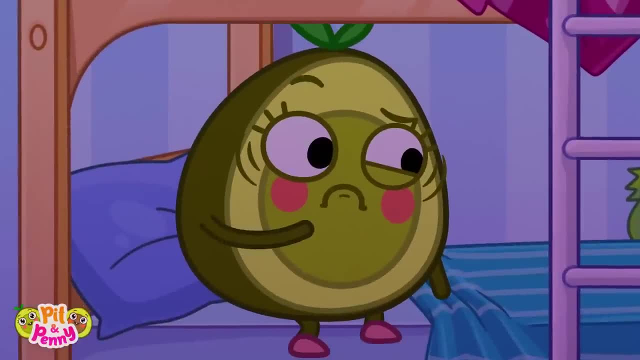 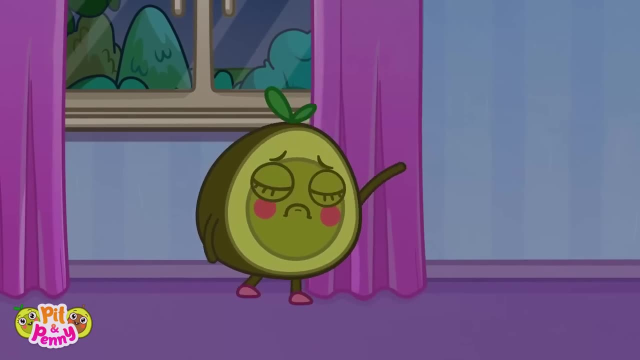 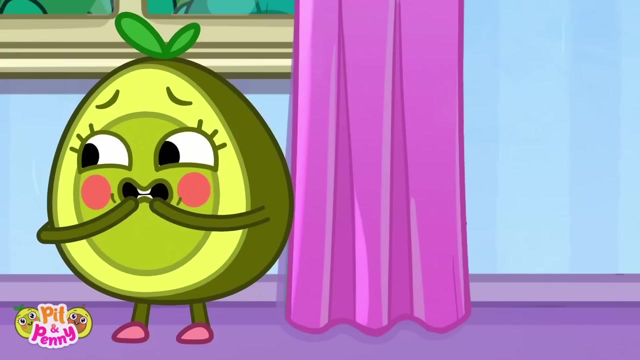 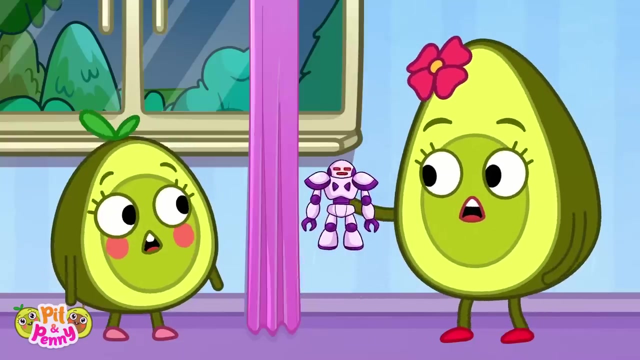 Penny, don't scare your brother. Give Mommy the ghost. What's that noise, Penny? It's coming from the window. Be careful, Penny. What's happened? Penny, It's just Pit's toy robot See, Nothing to be afraid of. 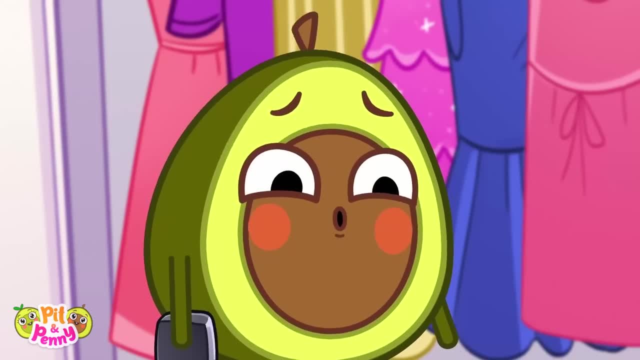 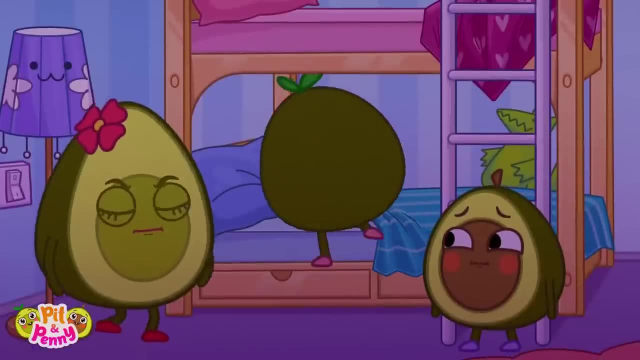 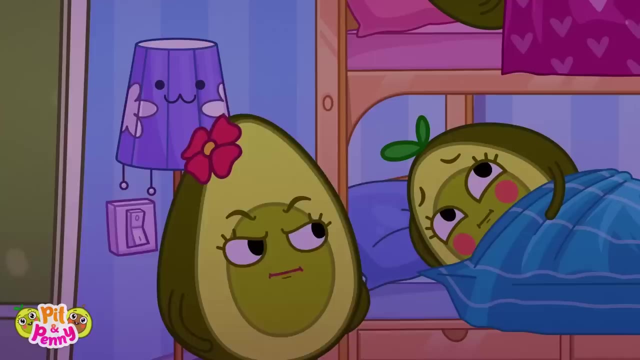 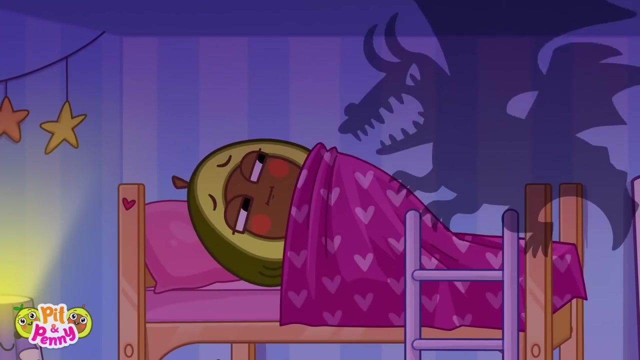 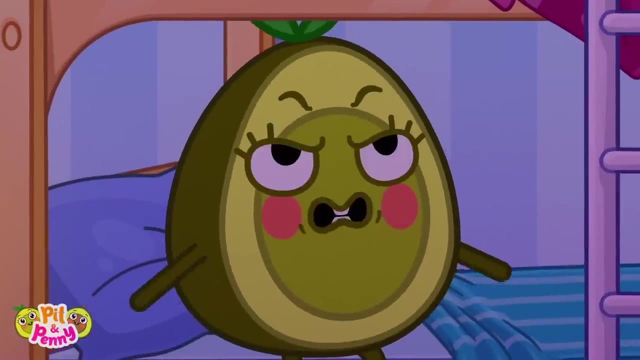 Stop scaring each other. Okay, Pit and Penny, back to bed. Come on, Pit, What It'll help you sleep. Is this another prank, Penny? I know it's you, What It's not me. Now, what could that be? 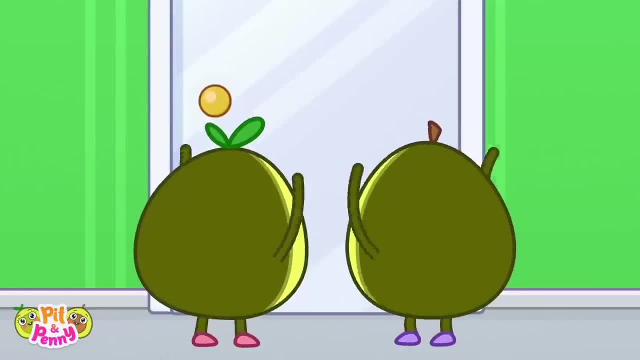 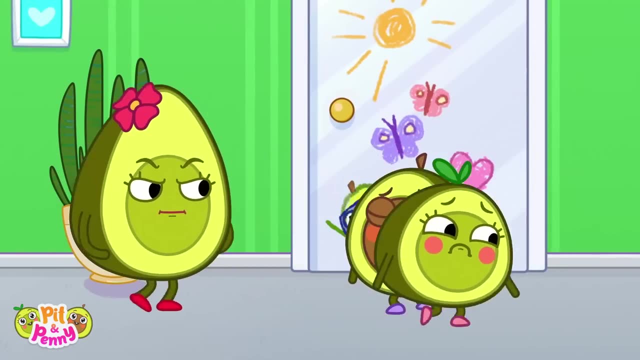 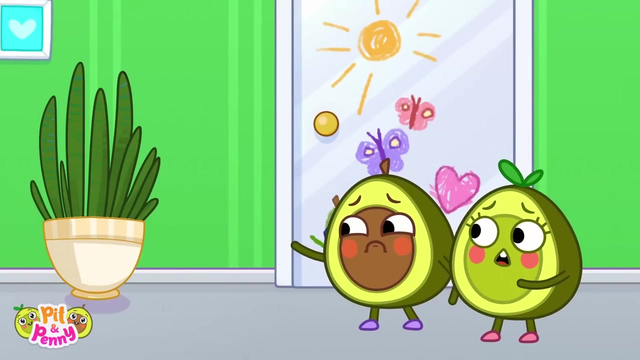 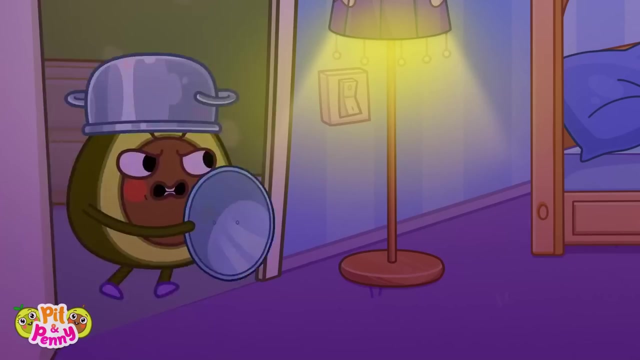 What? There's a monster in our room. Mommy thinks Pit and Penny are playing again. I told you to stop scaring each other. Go to sleep. They'll have to solve this on their own. Be brave Pit, Be brave Penny. 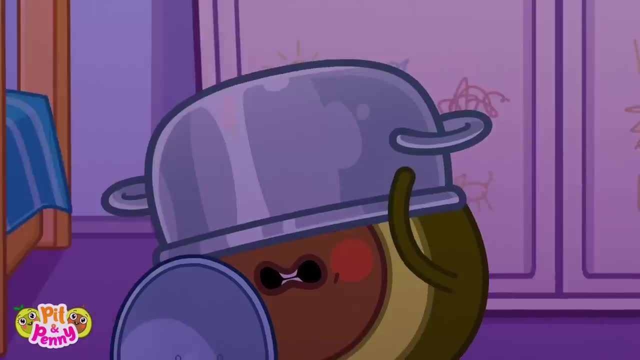 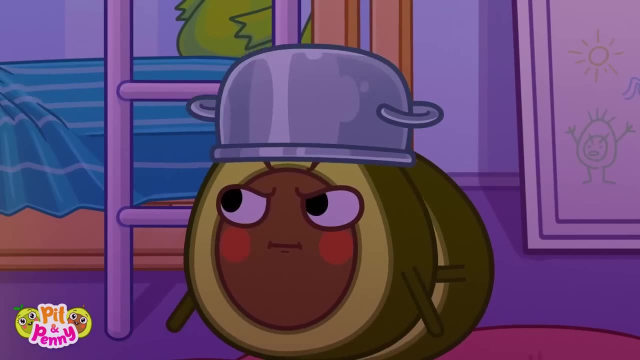 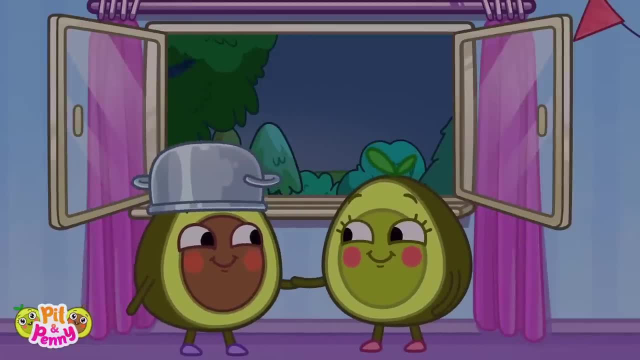 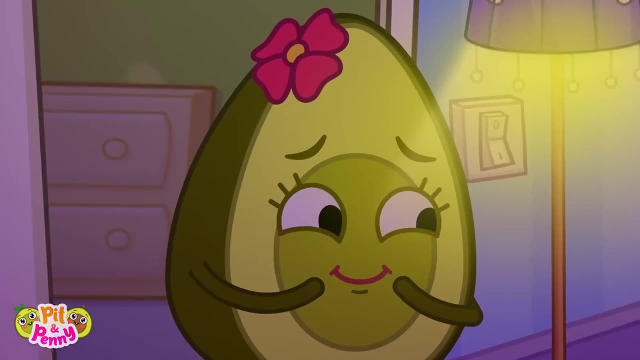 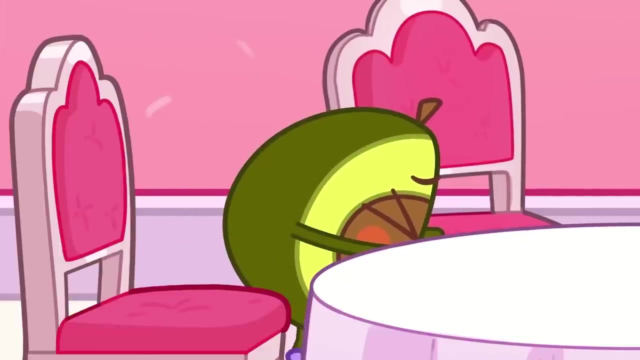 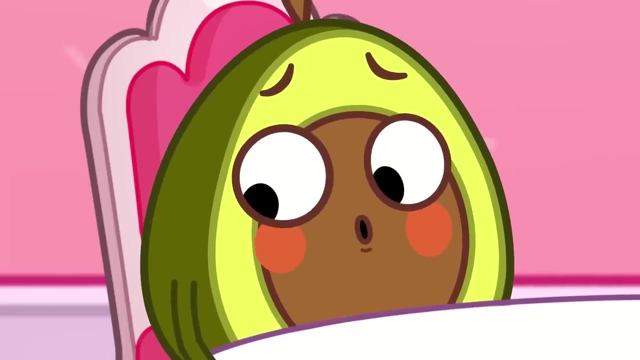 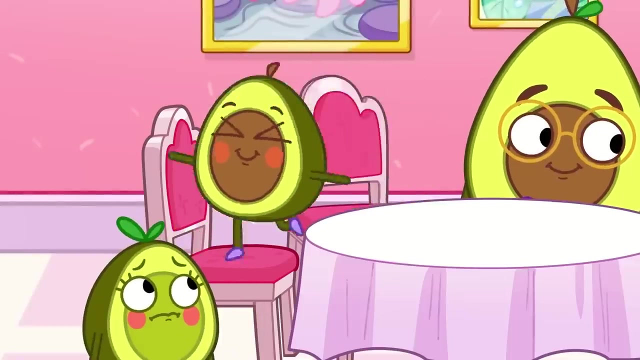 I'll never scare you again. Me too. See, Isn't that better? Pit and Penny are going to a fancy restaurant. Everybody find your seats. Pit found his. Your turn, Penny, Penny. Penny's seat is too high. No, Pit, don't play on the chairs. 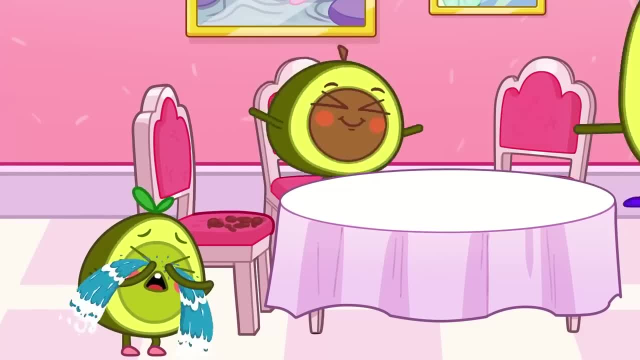 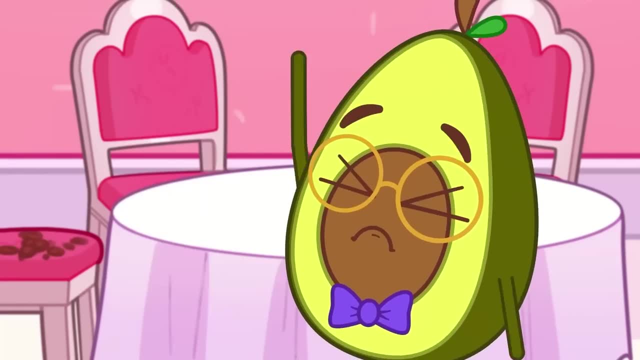 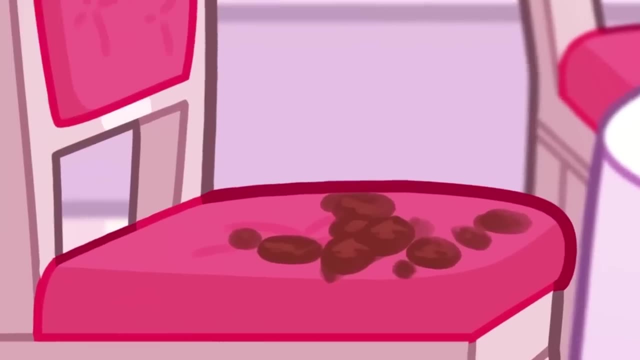 Look what you've done to Penny's feet And you might get hurt. Phew Daddy to the rescue. Pete, you shouldn't stand on a chair Now. how will you get out of here? Ah, Ah, Ah Ah. 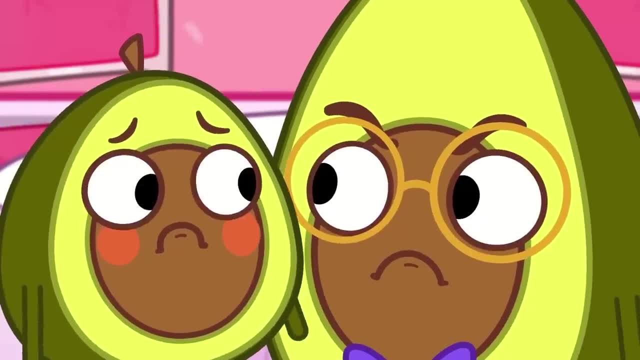 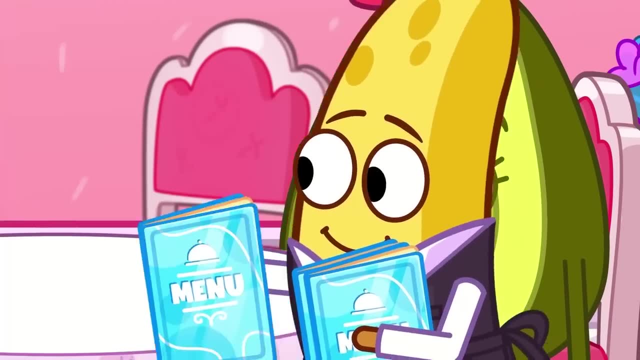 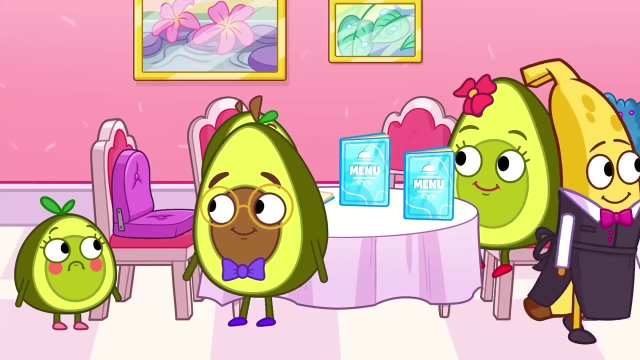 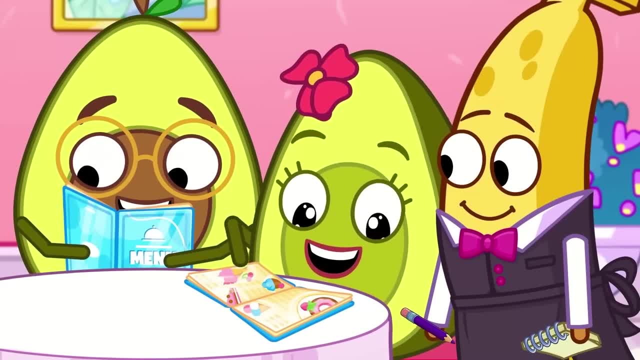 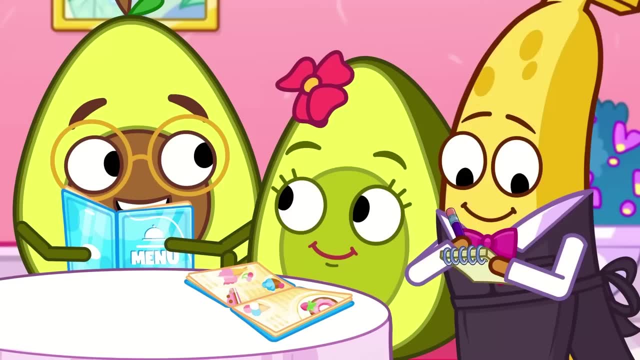 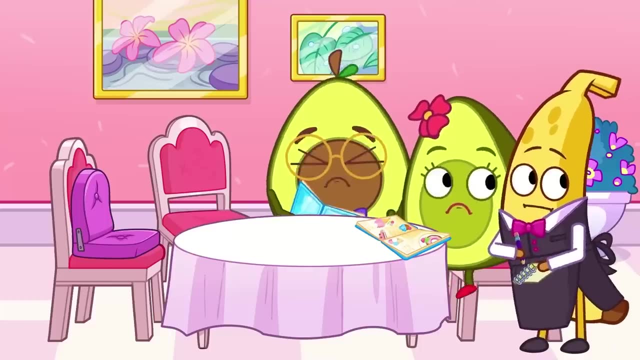 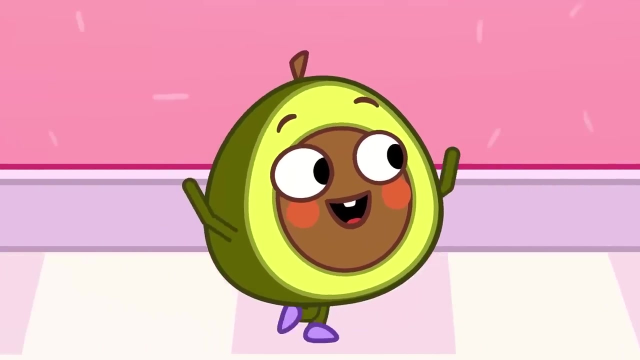 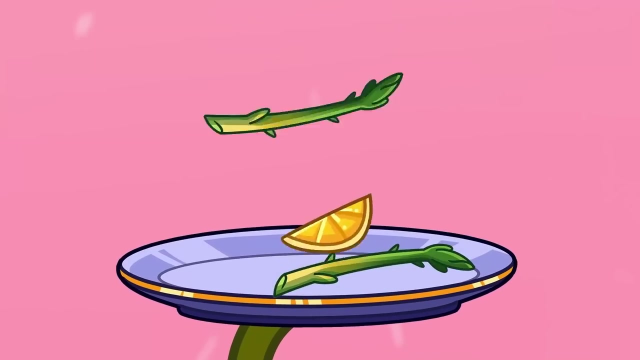 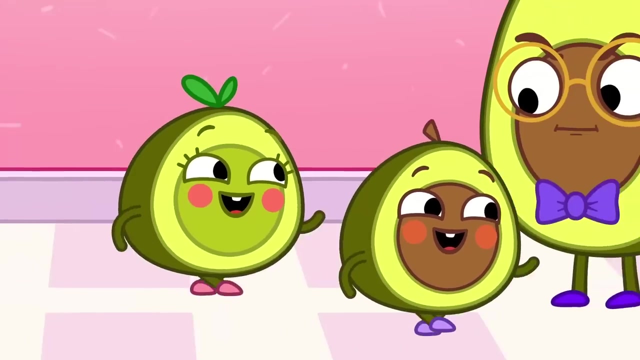 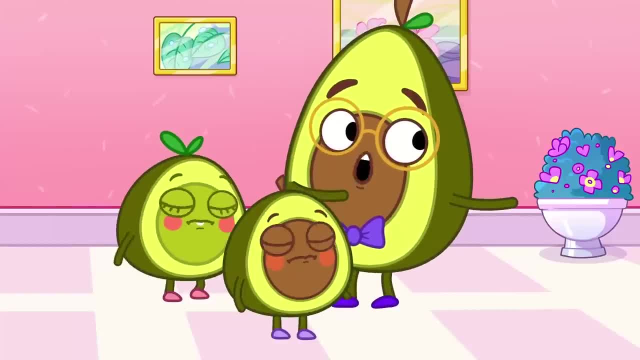 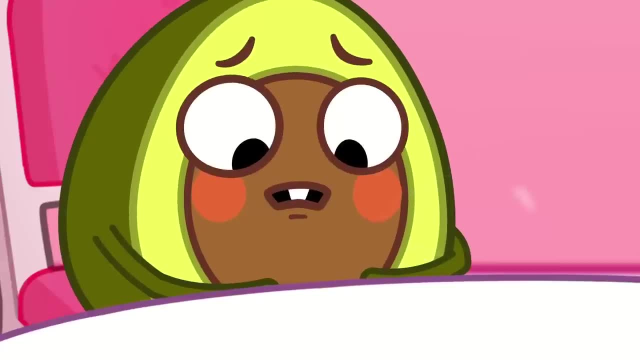 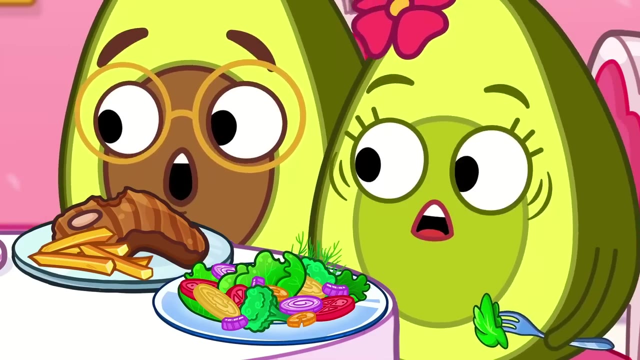 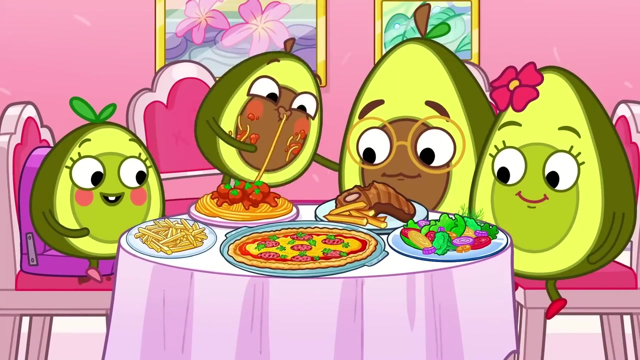 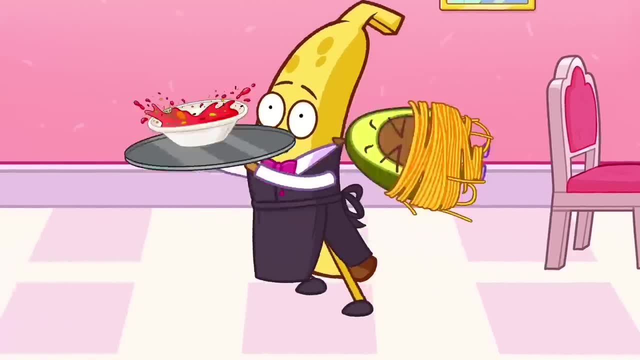 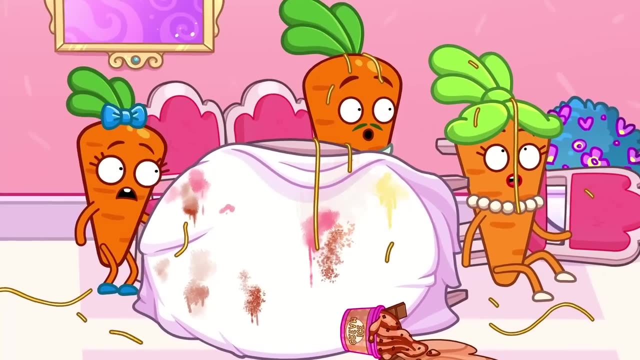 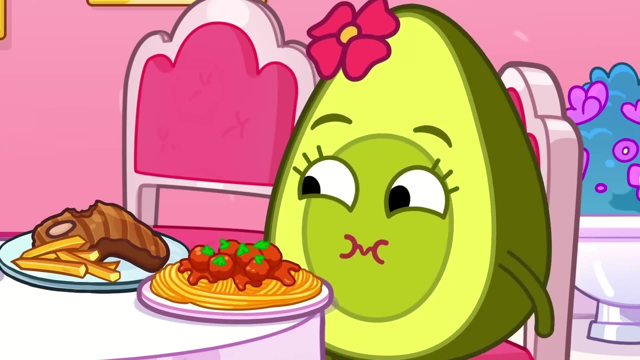 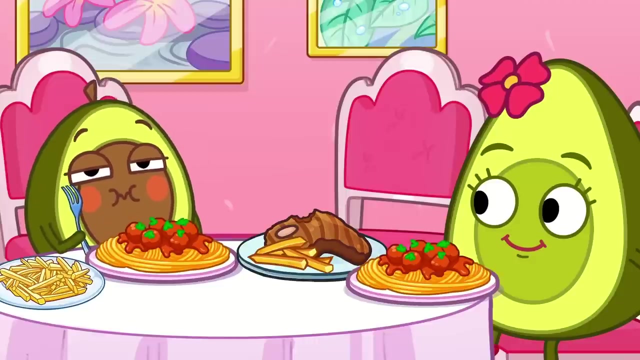 Oh, no, Kid is tangled up in his spaghetti. Oh, Oh, What a mess. Whoops, This is the proper way to eat. Now you try Pit Kids. you should follow the rules of conduct in the restaurant. Aww. 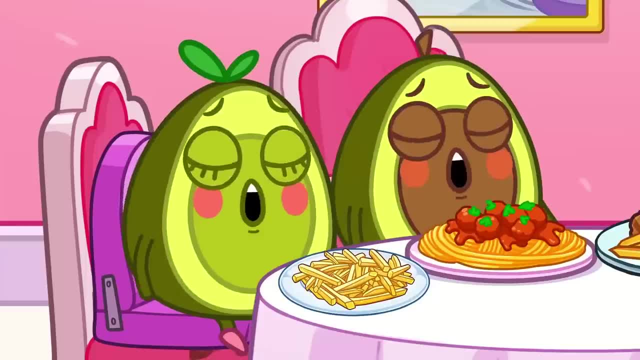 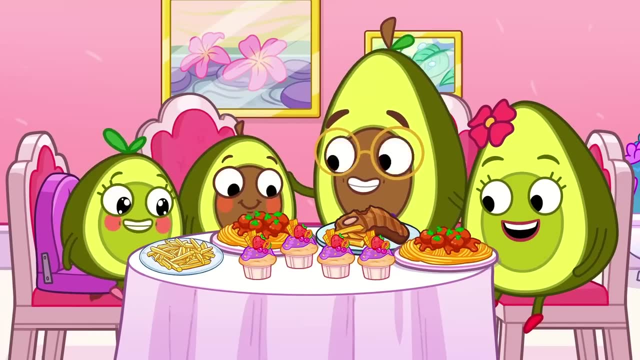 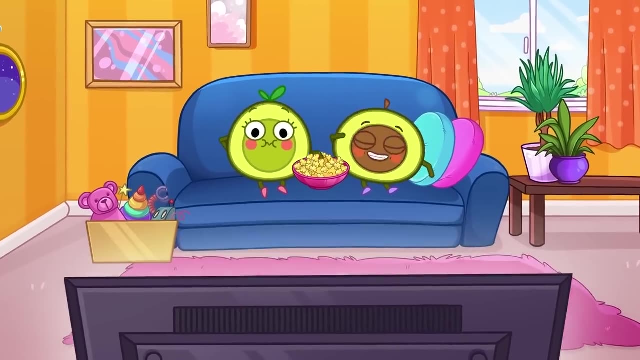 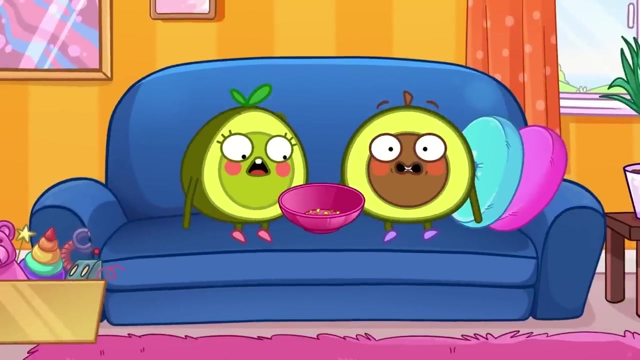 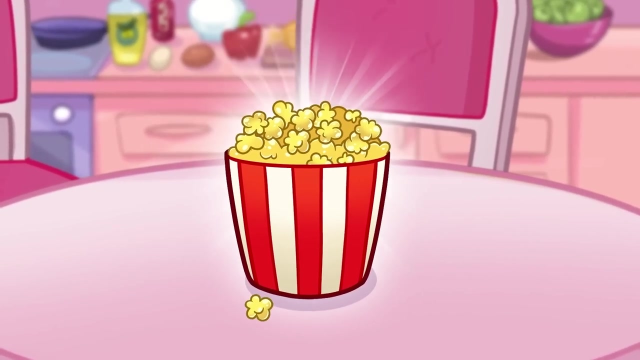 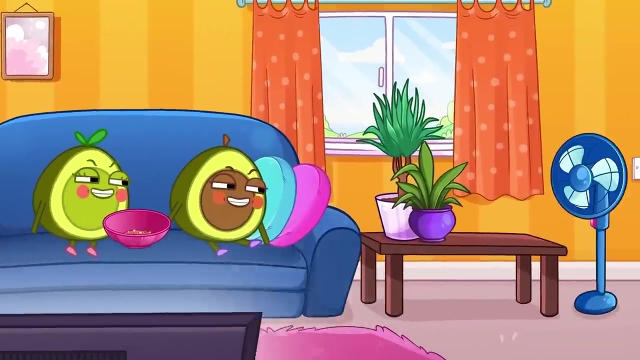 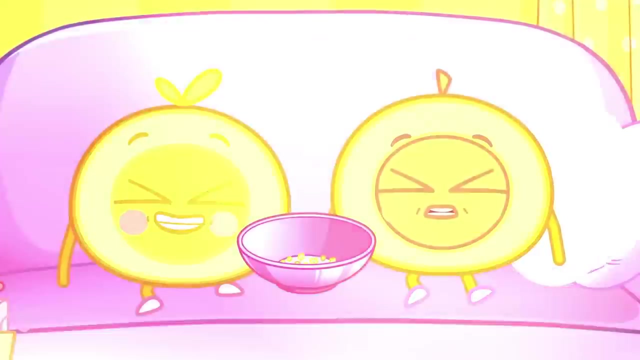 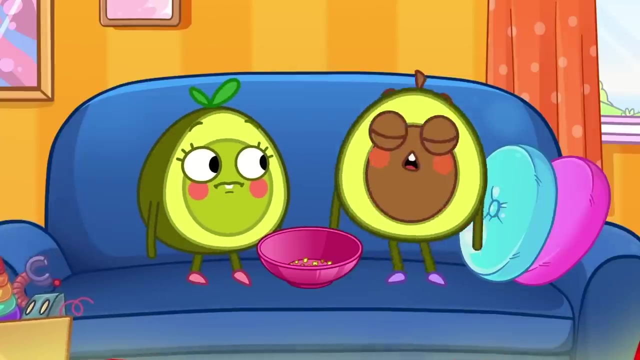 in the restaurant and look what daddy brought. bon appetit, hit and penny love eating popcorn, but now the bowl is empty. maybe there's more in the kitchen- challenge time. what kind of game will pit and penny play? oh no, the floor is now molten lava. who can get to the popcorn first without touching the floor? 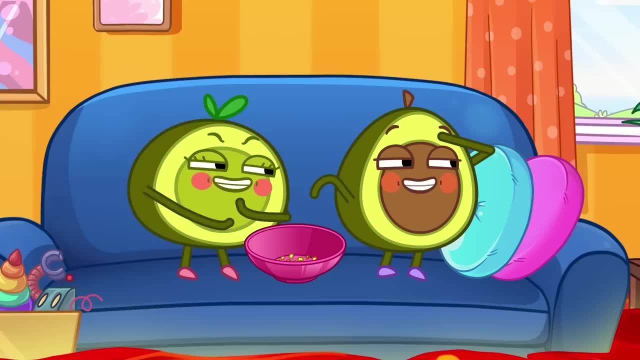 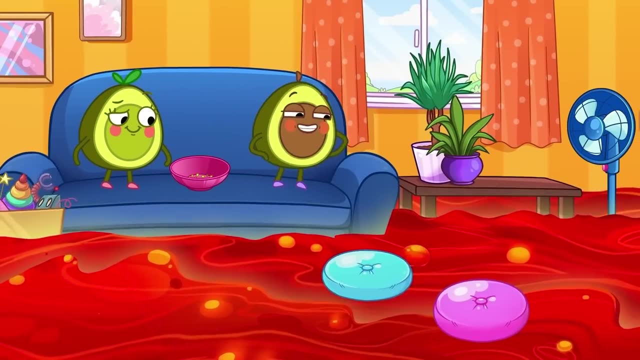 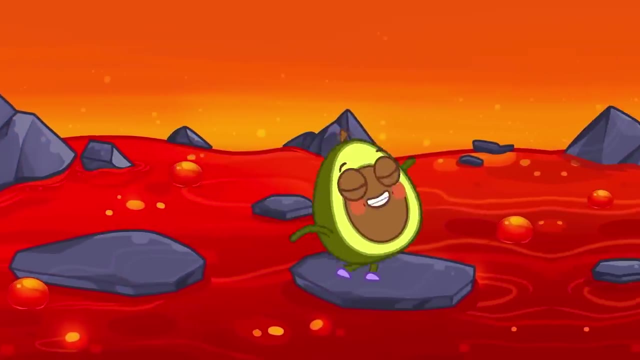 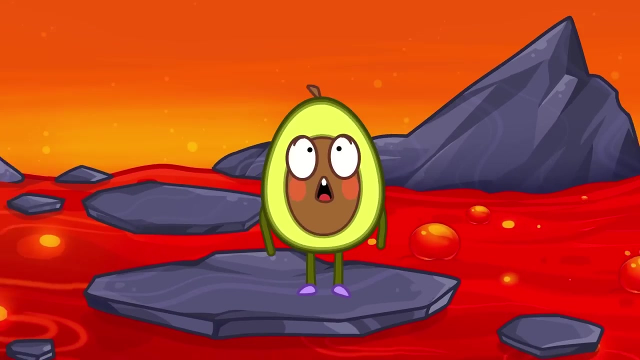 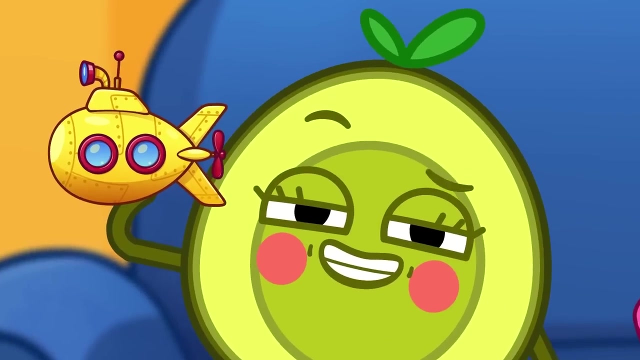 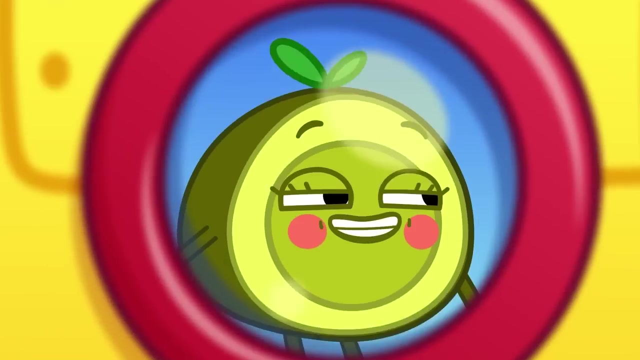 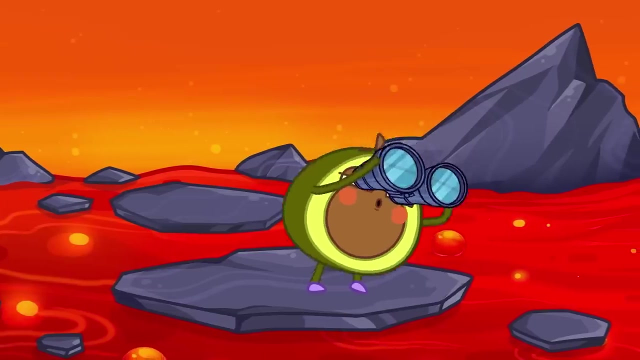 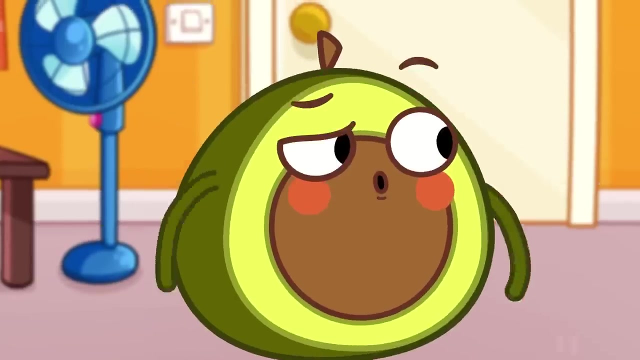 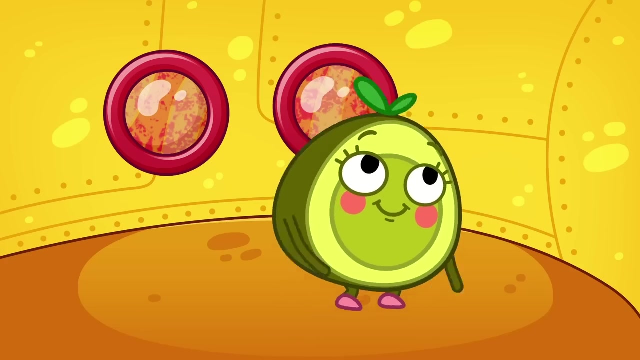 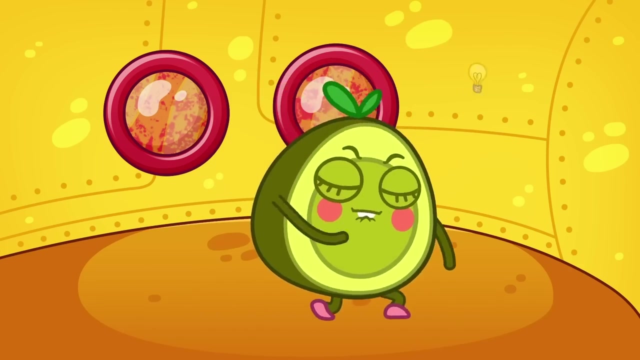 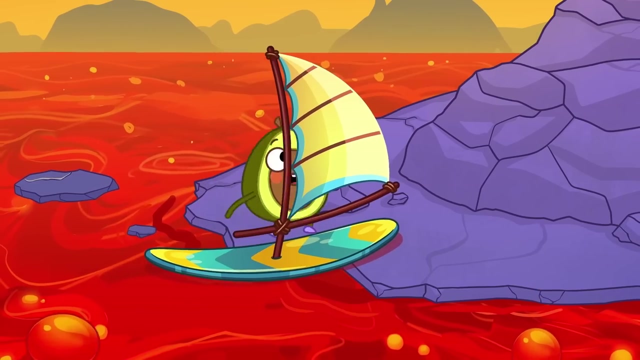 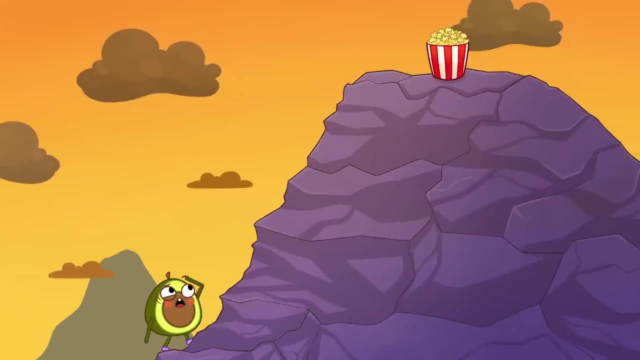 it uses pillows as rocks. the popcorn is still so far away. penny thinks a submarine will be faster. go, penny, go. oh how, what will you do bad? maybe penny can use those building blocks just a little bit further and pit will win the race. but the man can't win a race. 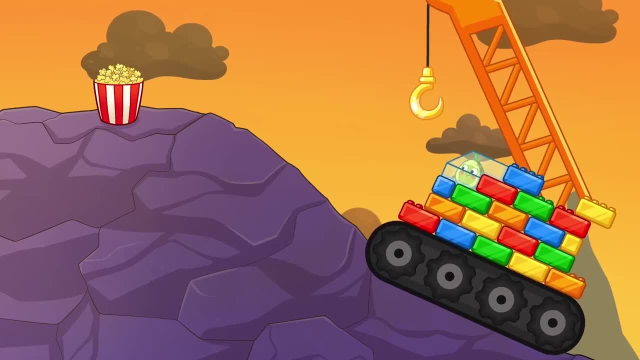 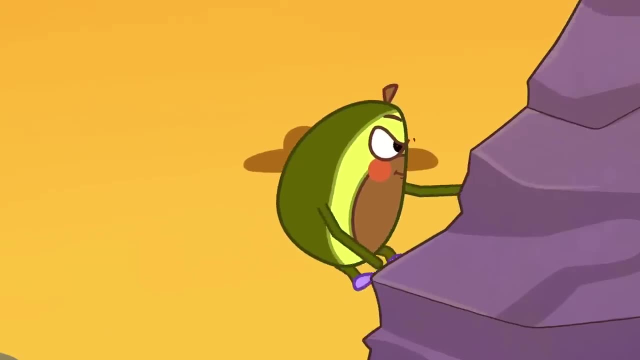 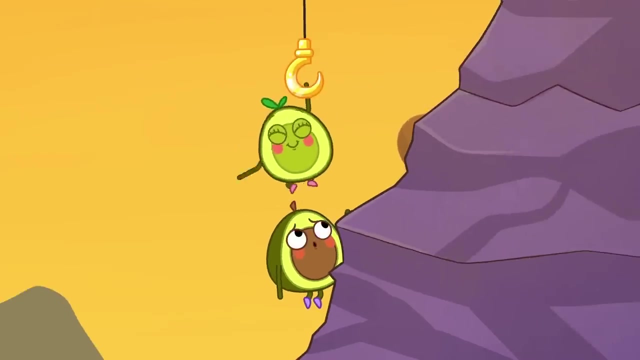 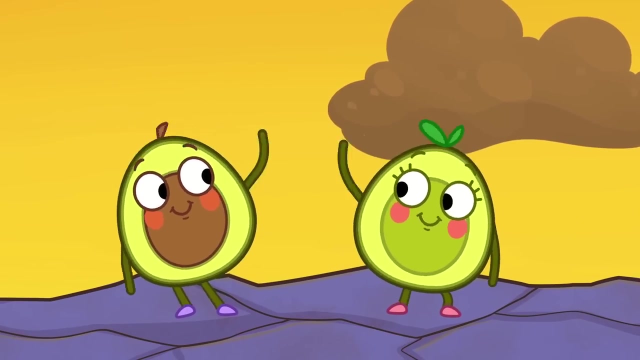 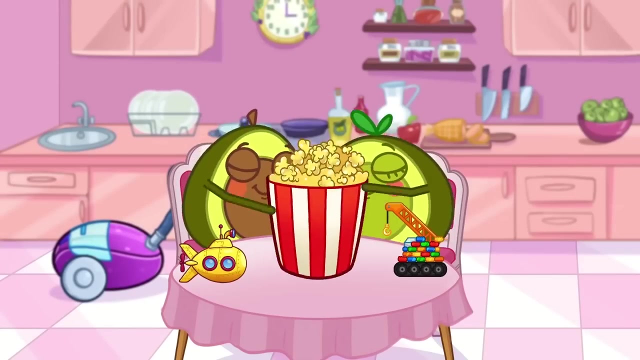 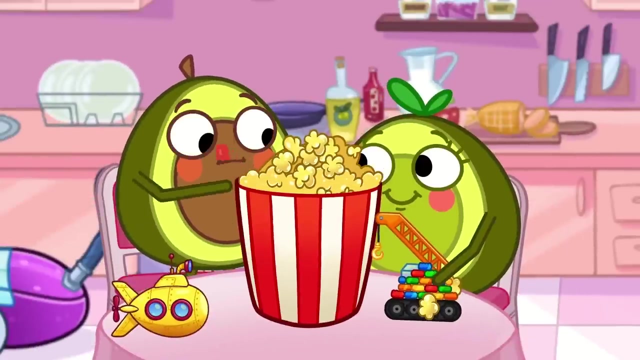 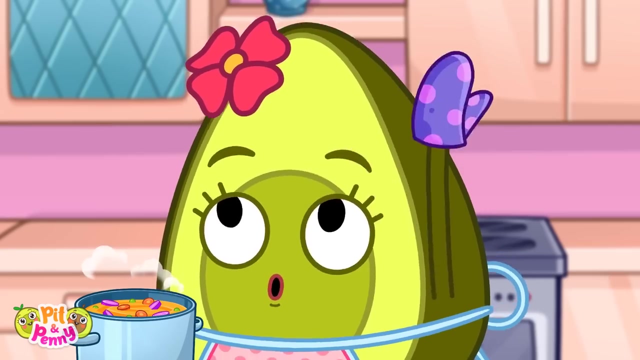 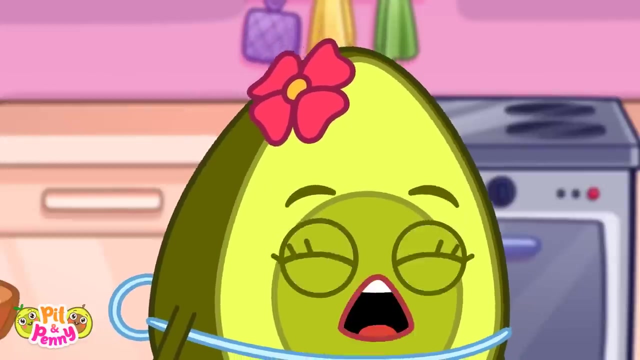 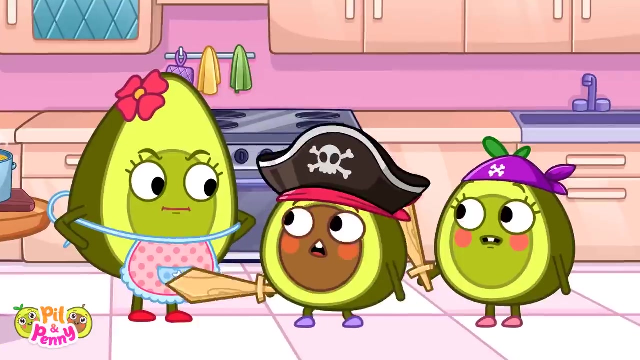 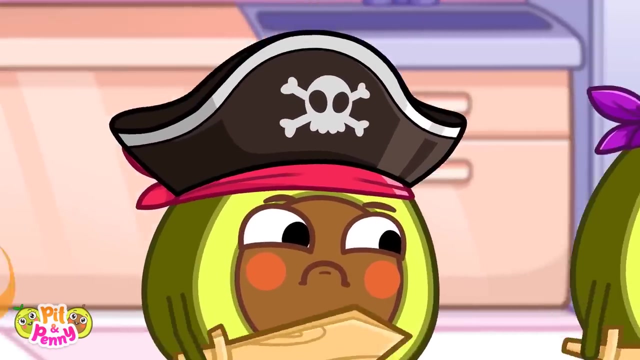 but the man can't win a race mountain is very steep and very dangerous. careful bit, hold on. penny is coming to rescue you and the popcorn treasure. enjoy your yummy treat. mommy is busy in the kitchen and pit and penny are playing pirate. this isn't the best place to play. the kitchen is no place for pirates. sorry pit, sorry penny. 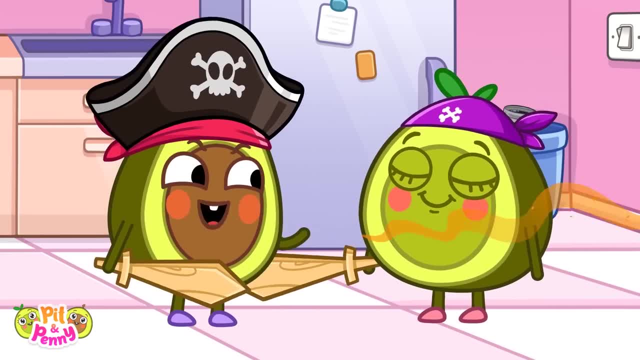 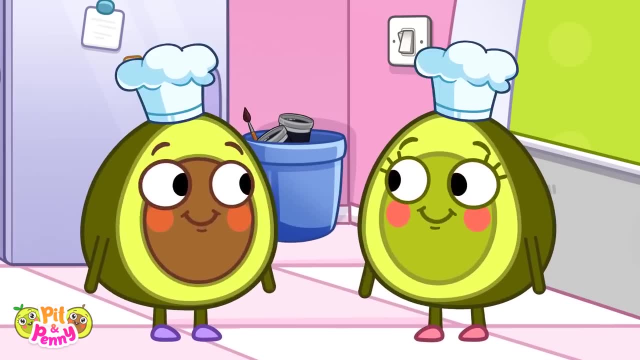 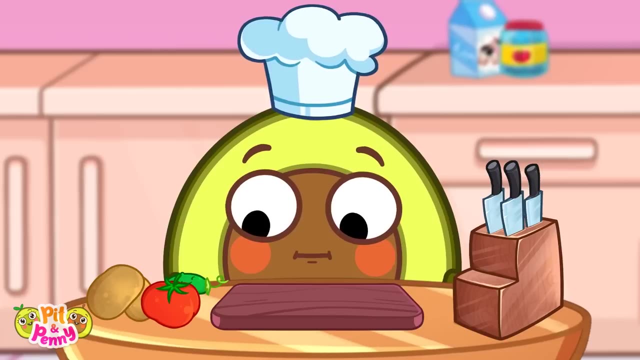 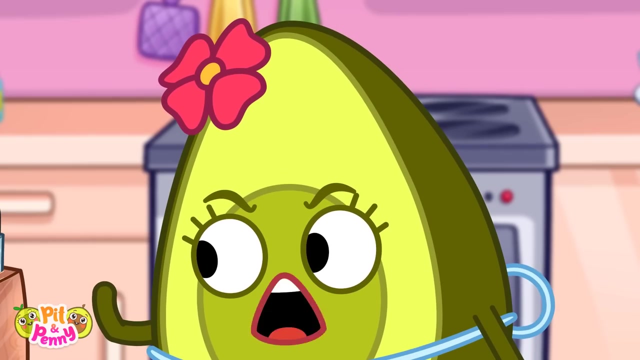 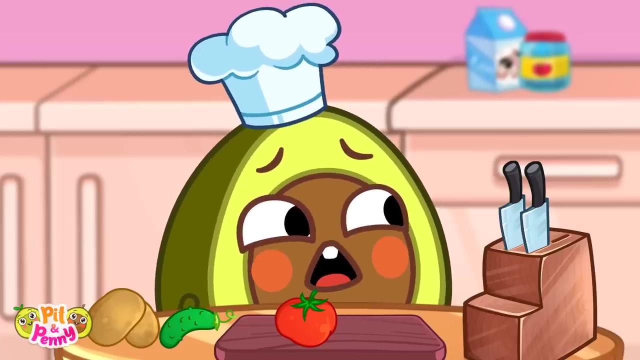 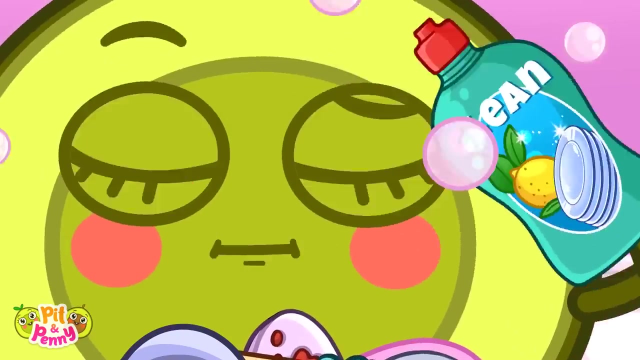 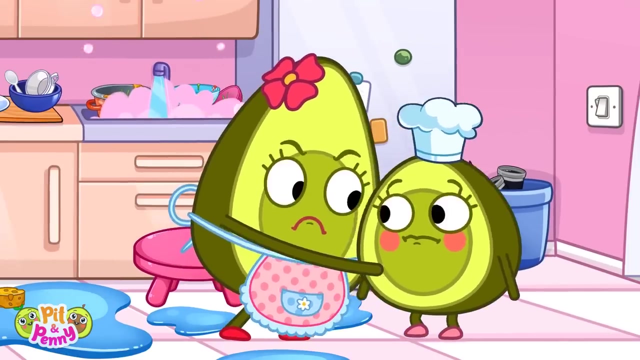 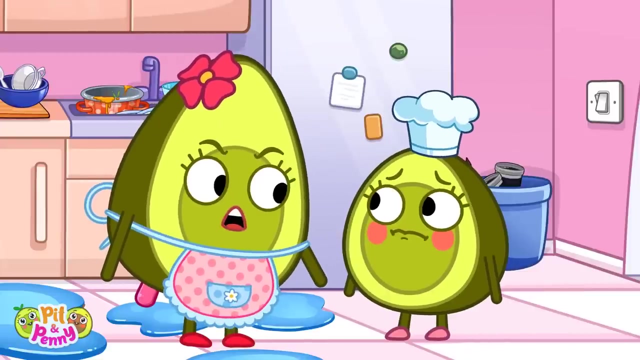 what a place now. pit and penny want to help mommy in the kitchen. careful, pit, those aren't toys. no pit. children shouldn't use sharp objects. i'm sorry, what's penny up to? oh, penny, there's already soap in the water. oh no, in the kitchen you always need to be careful and attentive. i'm sorry, where's pit? 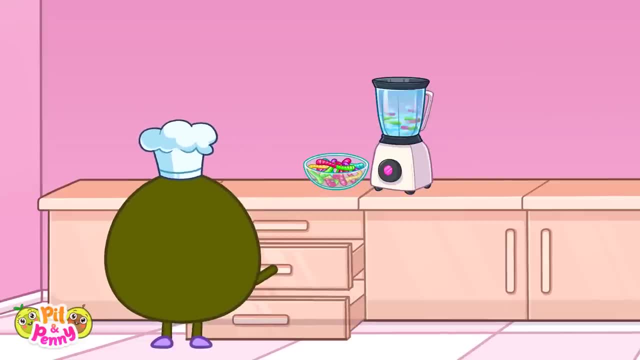 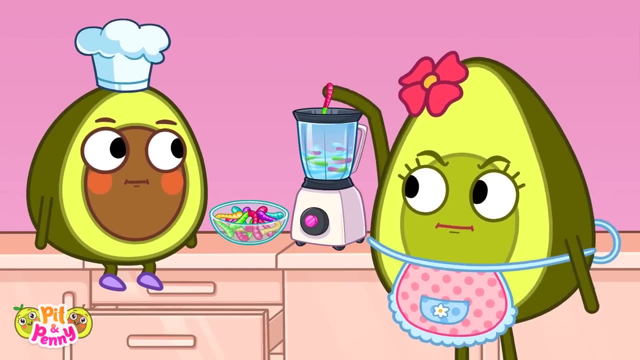 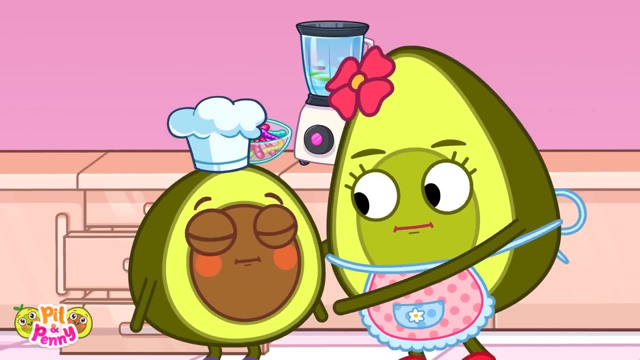 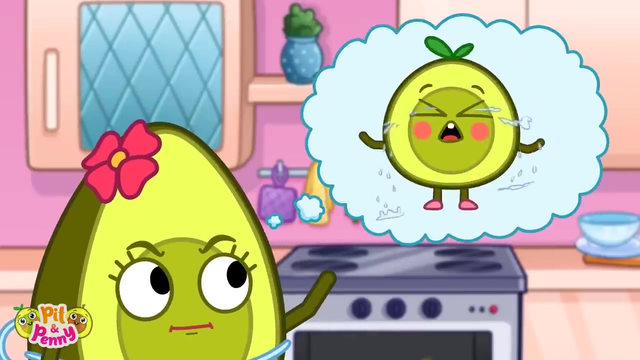 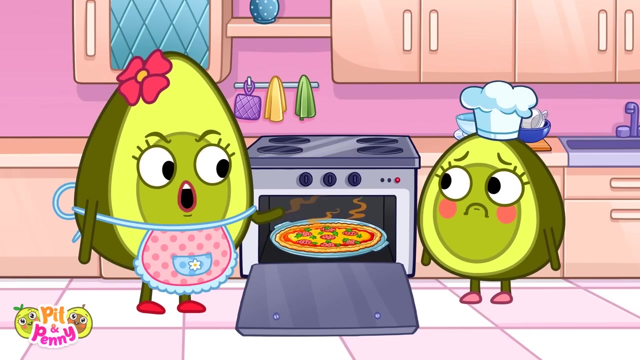 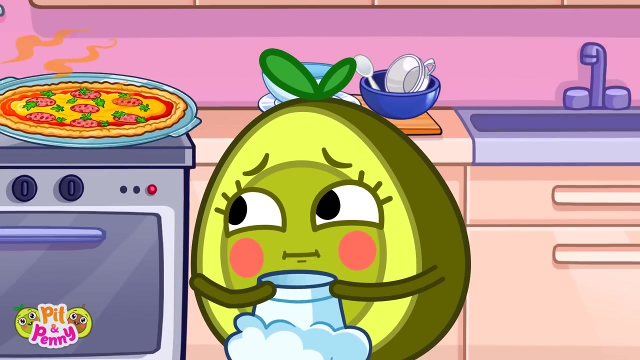 pit, you shouldn't be up there. working appliances are dangerous. i got it, mommy. mommy, maybe we should check on penny. careful penny. ovens are hot. okay, children shouldn't touch the oven. we just wanted to help you. is there some way to help you pit, and penny can help you. can be my kitchen alarm clock. 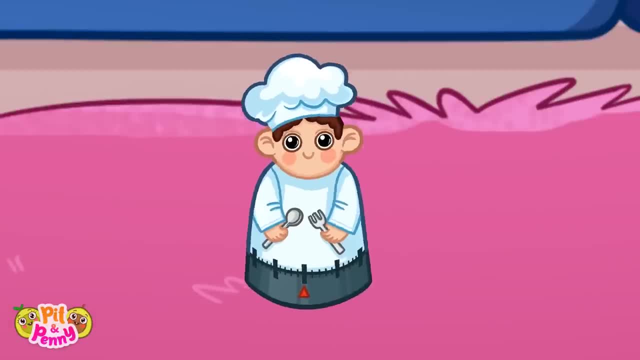 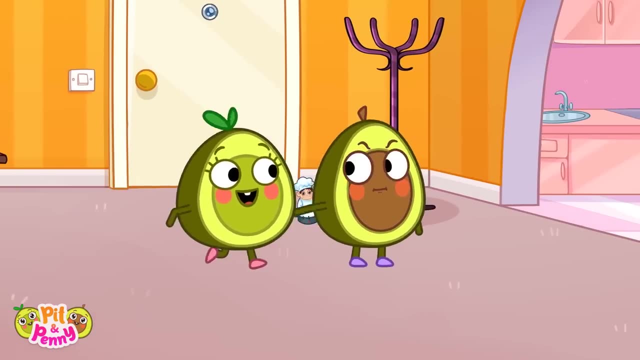 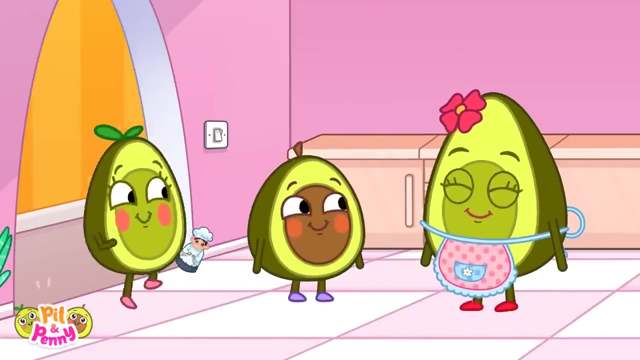 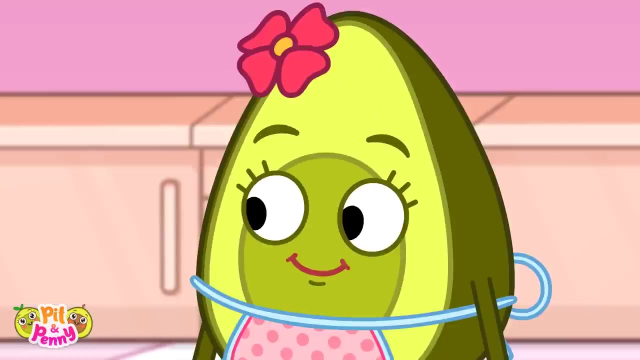 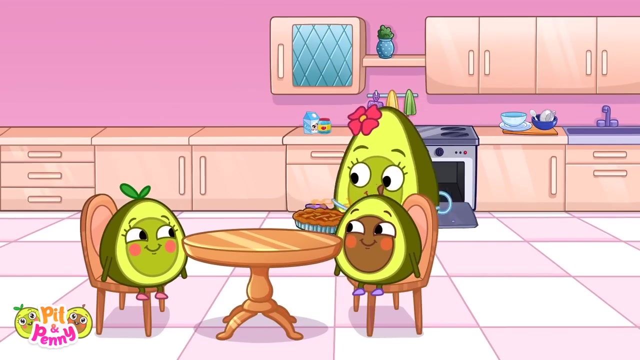 there's no running in the kitchen. lunch is ready. thanks for the help. you can be my kitchen alarm clock. yay, lunch is ready. there's no running in the kitchen. let's go to help kids. yum, mommy baked a pie. now you know how to behave in the kitchen. 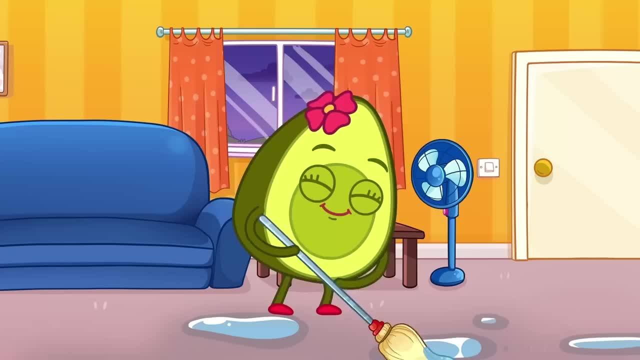 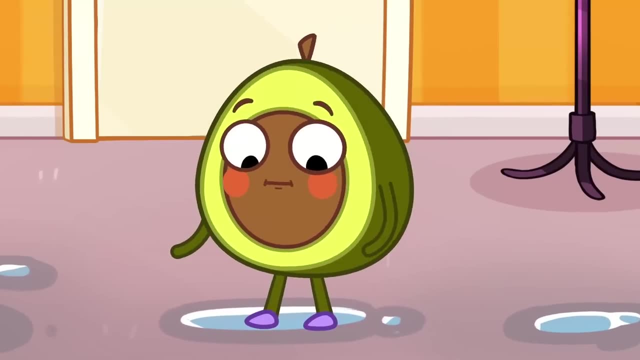 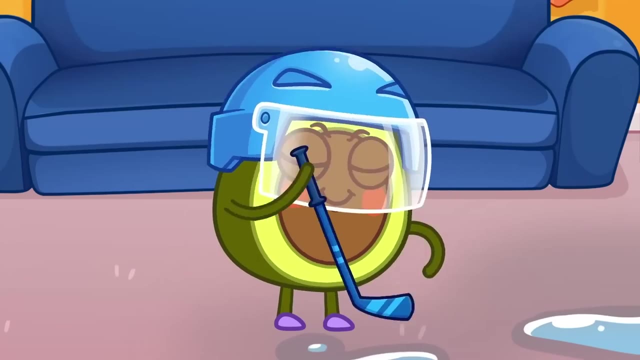 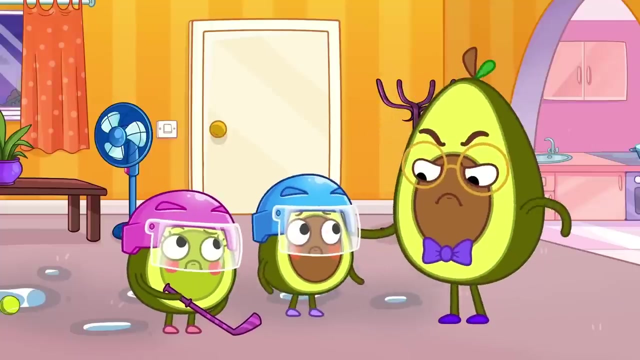 mommy is busy cleaning the living room. careful you might slip. what are you thinking, pit? hmm, you shouldn't play with the kitchen door. you shouldn't play with the kitchen door. you shouldn't play hockey inside. good thing daddy was there to catch you. kids, don't play on the wet floor, it's. 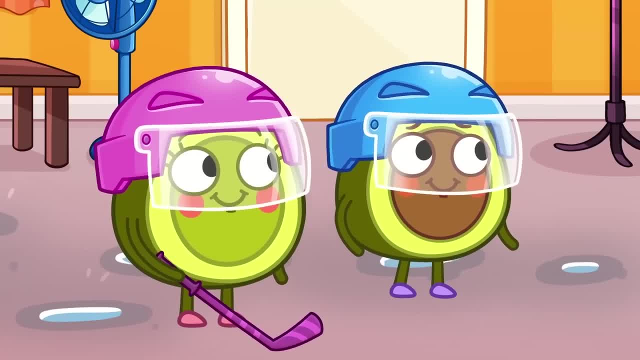 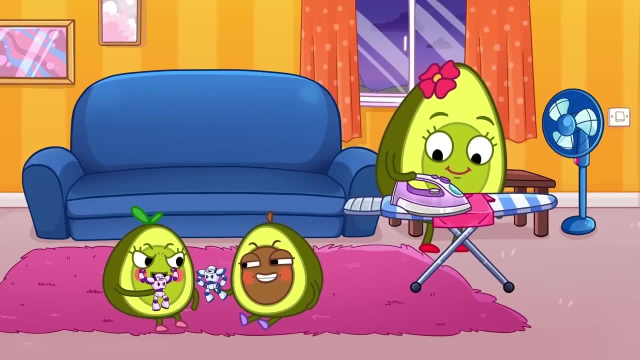 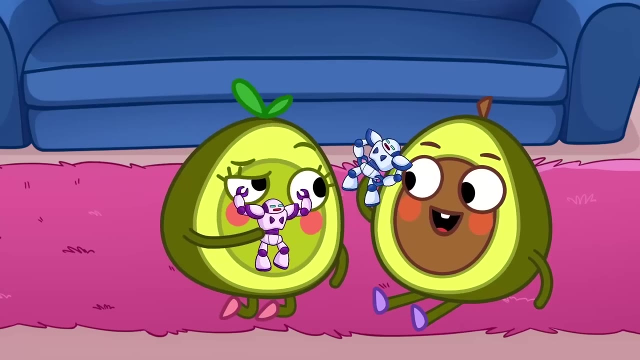 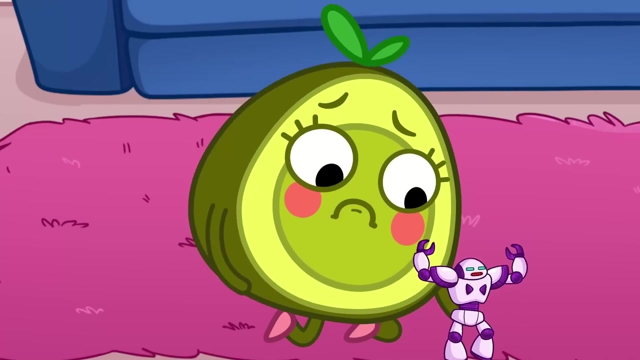 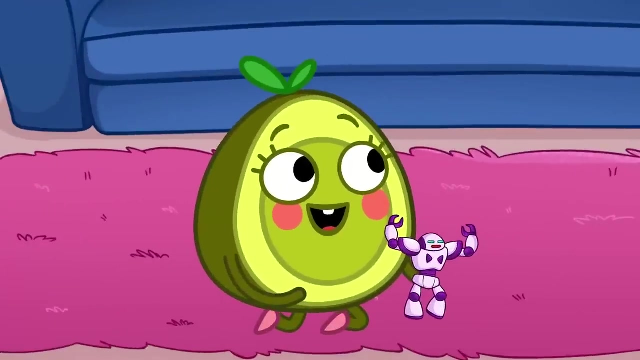 kids don't play on the wet floor. it's dangerous pit and penny are now playing with their pit and penny are now playing with their robots. but penny's robot doesn't have a. They brought rock snow. sorry, penny, the iron is not a toy. sorry, penny, the iron is not a toy. 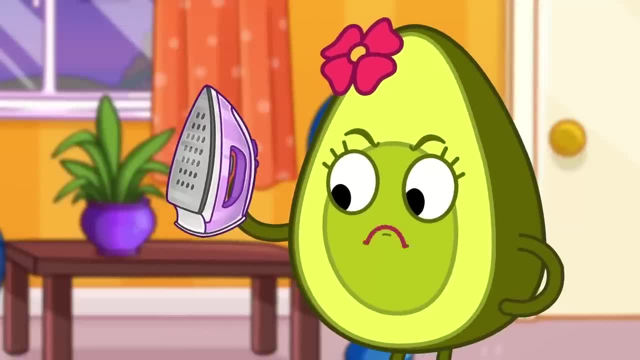 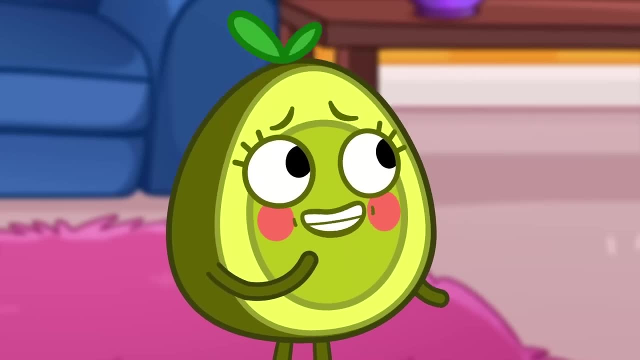 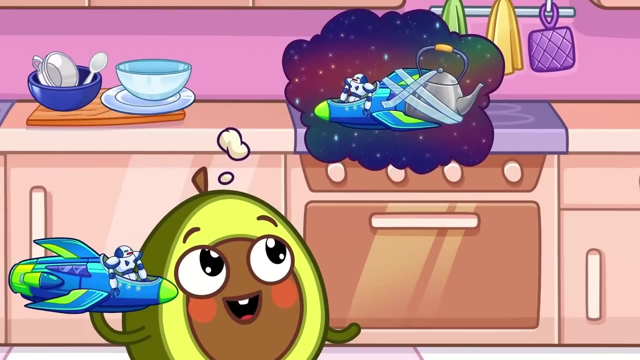 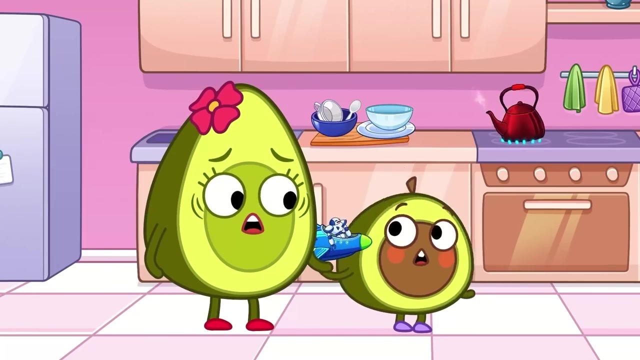 oh, penny, don't touch the iron, it's still hot. you, uh, penny, don't touch the iron, it's still保护 hot brain. you don't touch the iron, it's still hot. No Pit, The kettle is not a toy. A kettle can be very hot and dangerous. 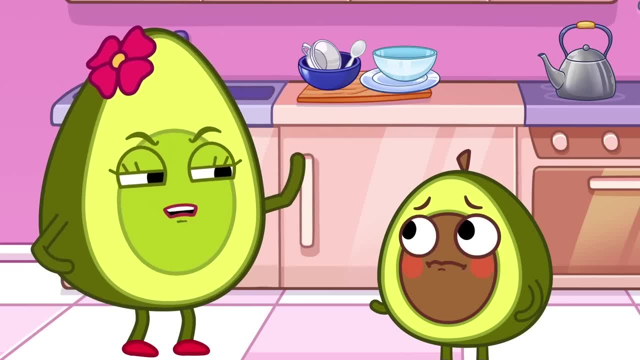 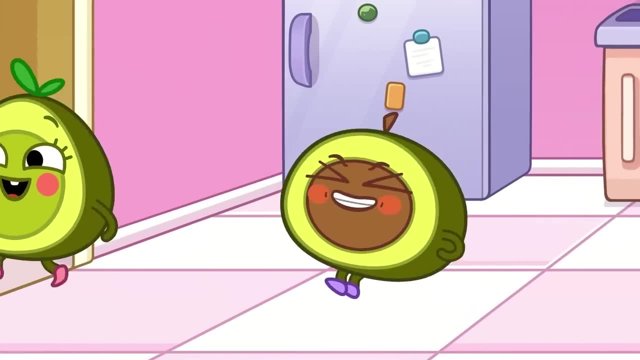 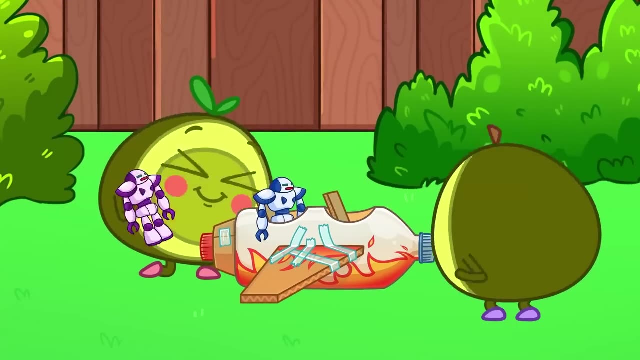 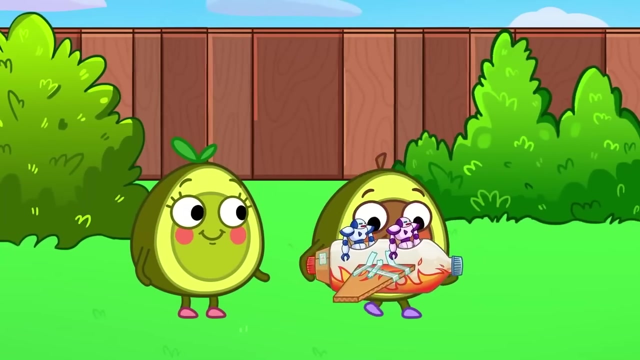 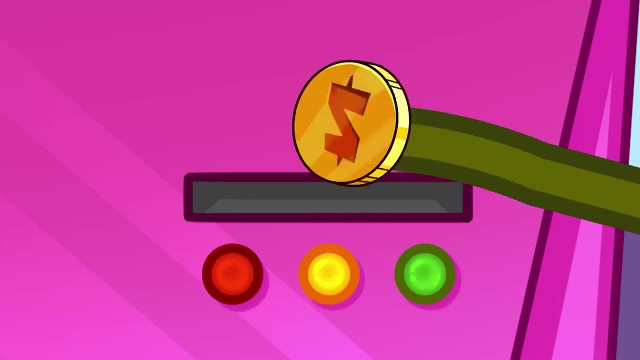 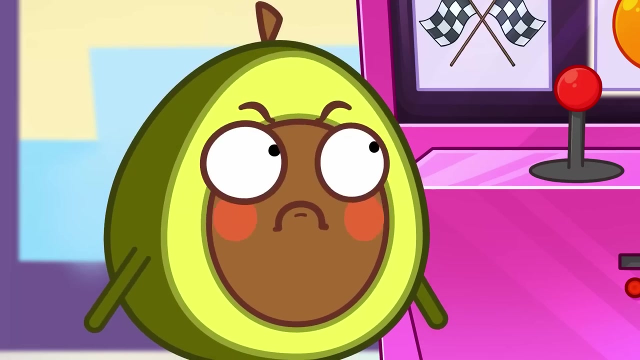 Pit, be careful with the kettle, You can be burned. There's now room in the rocket for both toys. Well done, Pit and Penny. Pit and Penny are playing a video game. Penny wants to play Munchman, But Pit wants to play Speed Racer. 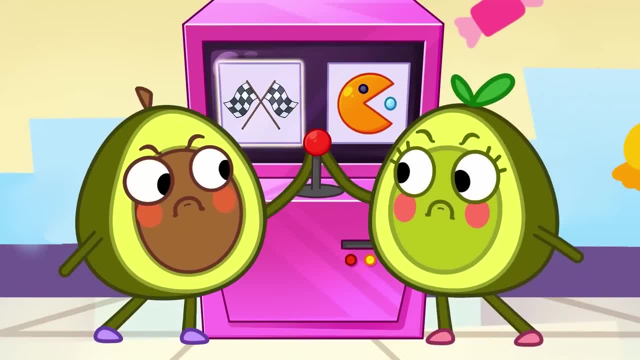 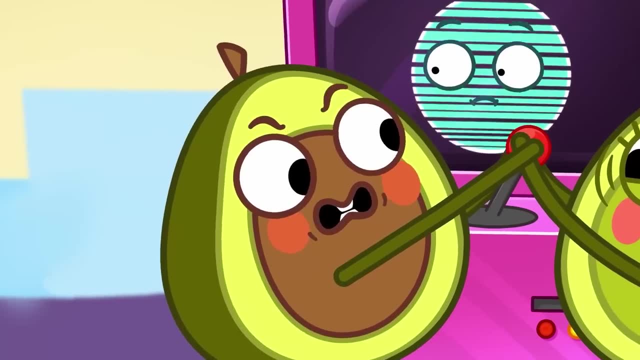 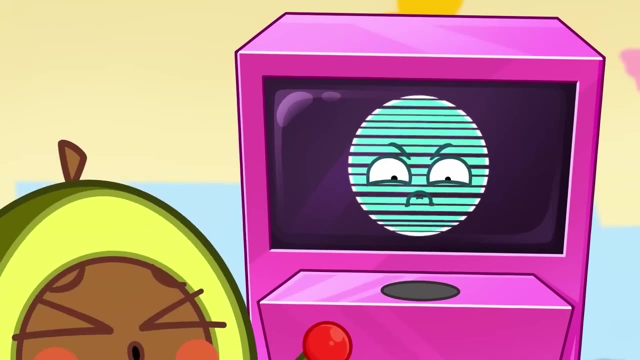 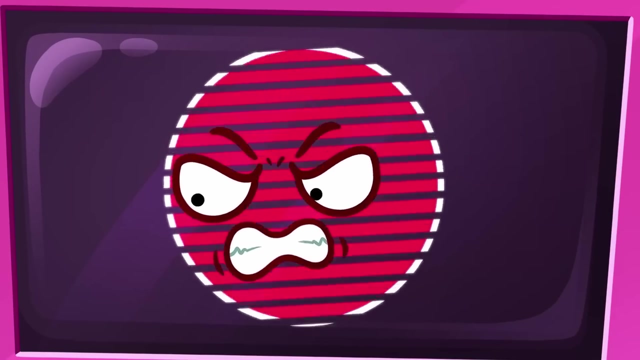 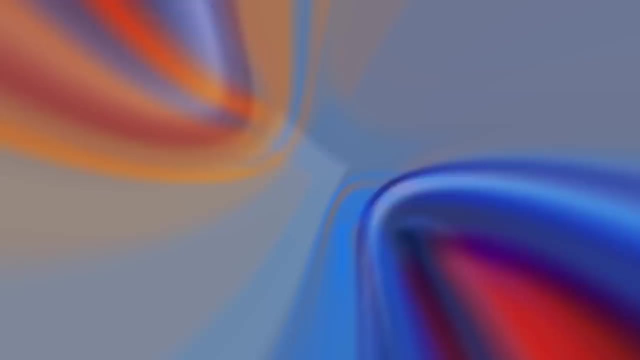 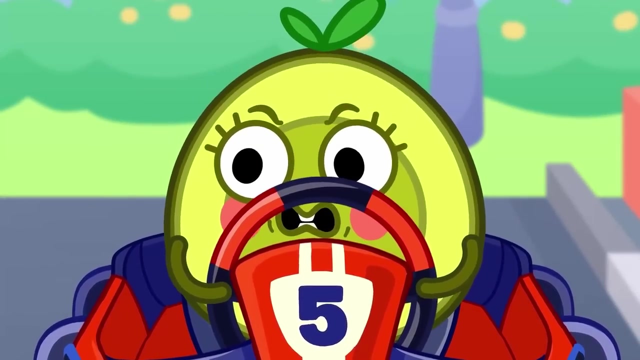 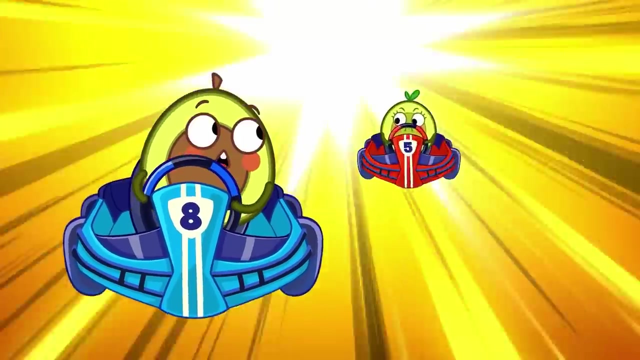 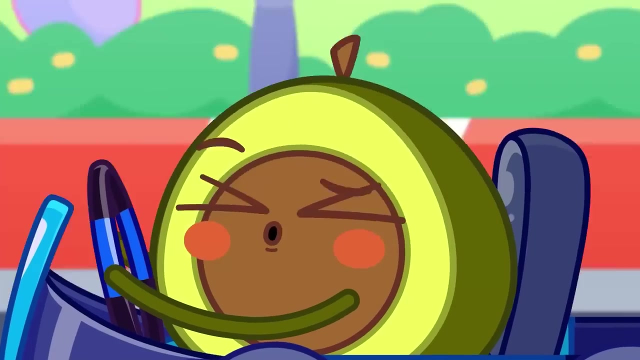 Be careful, kids. Now you've broken the joystick. The computer seems angry. Pit and Penny are inside the racing game. Hurry Penny Pit's winning. It looks like Penny's catching up. It's a power-up, Hehehehe. 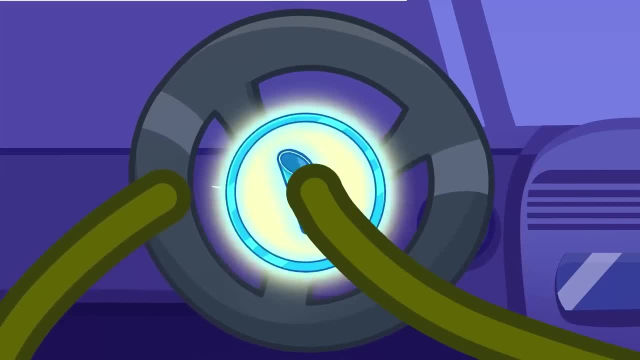 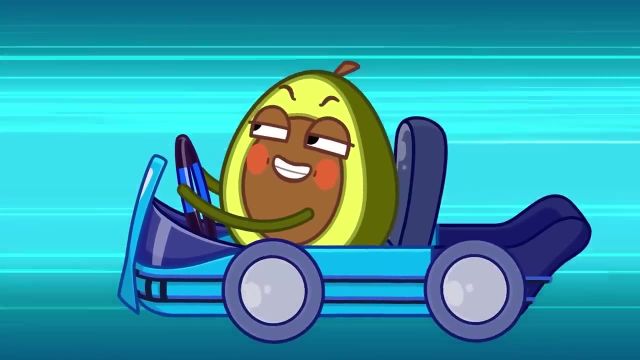 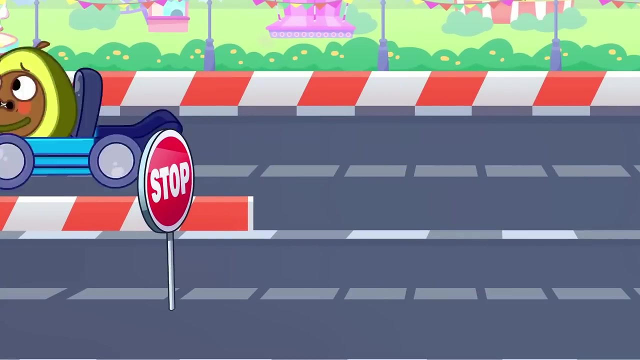 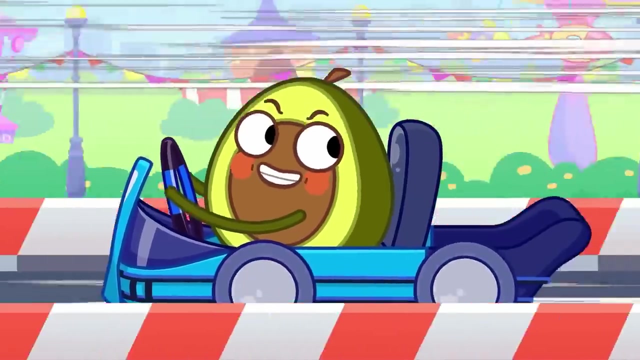 Hehehehe, Hehehehe, Hehehehe, Hehehehe. It was a smoke bomb. Hehehehe, You better stop Pit Huh. Ah, Wow, Hehehehe, Huh. 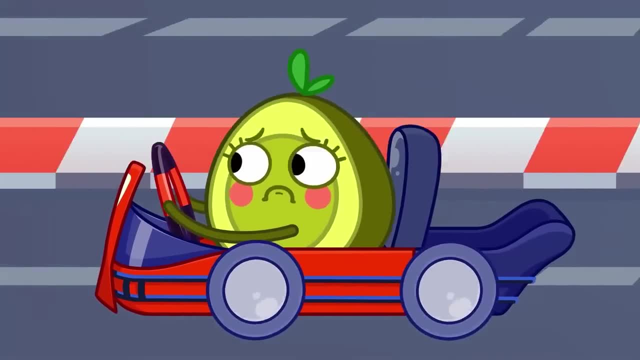 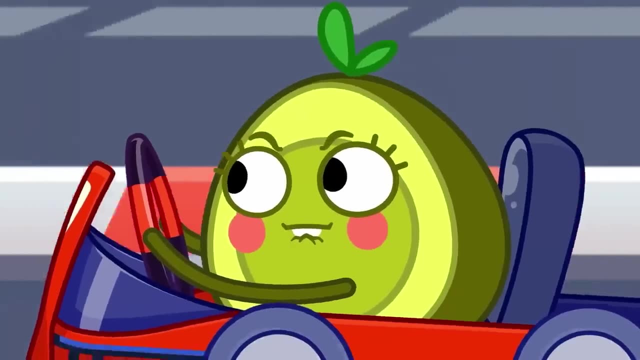 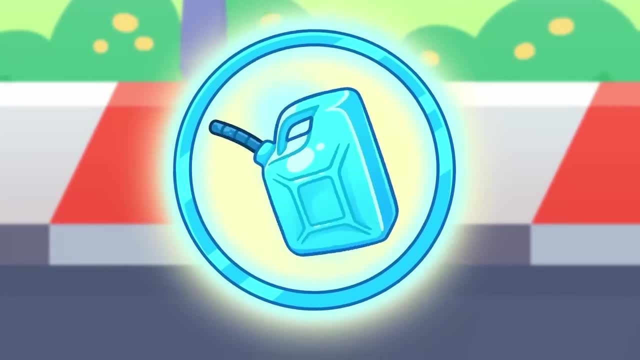 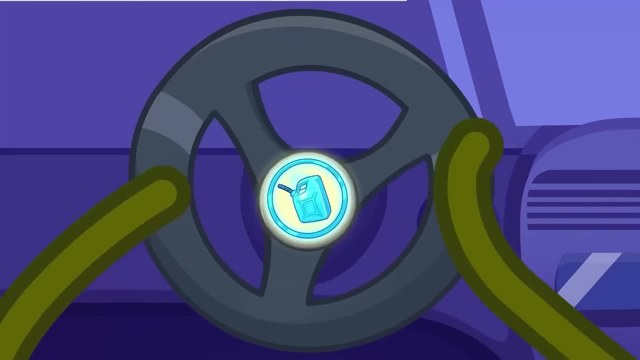 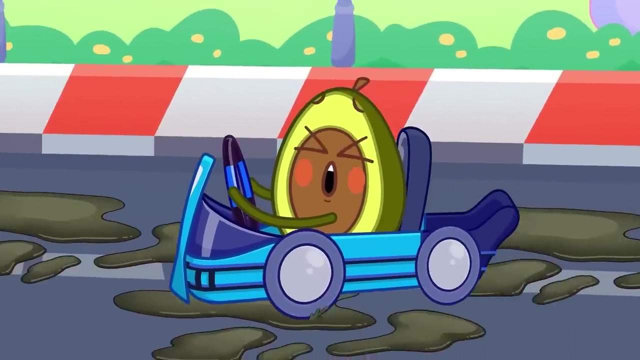 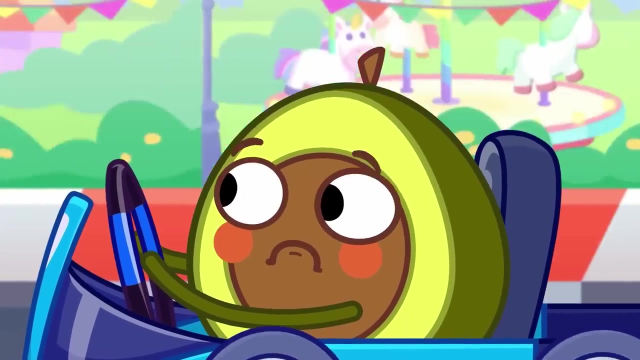 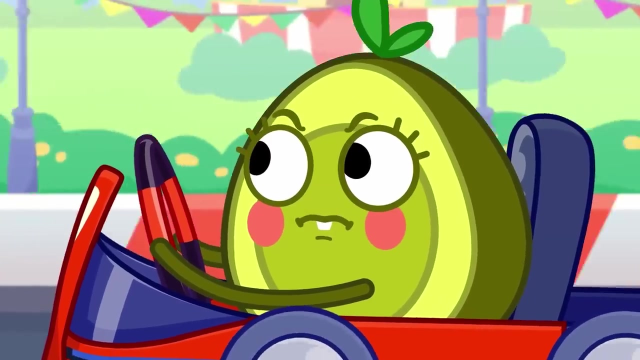 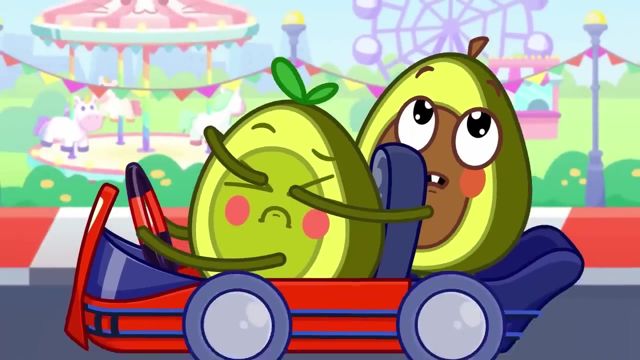 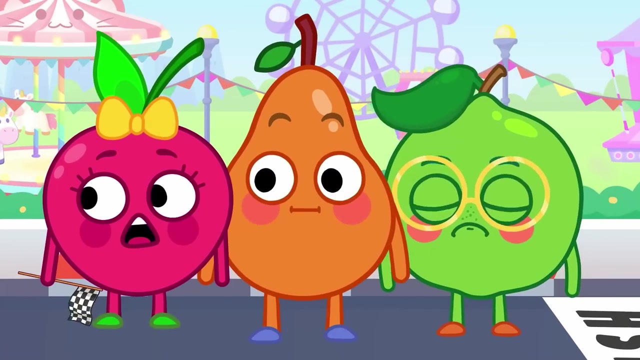 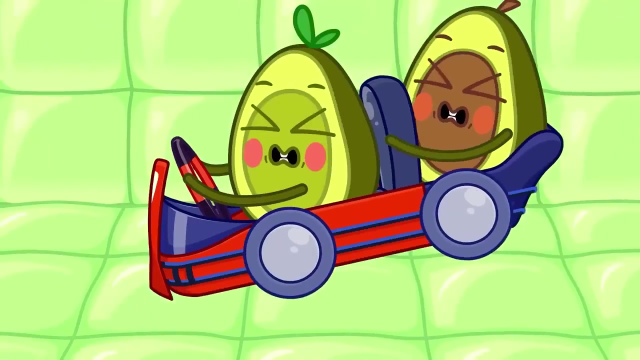 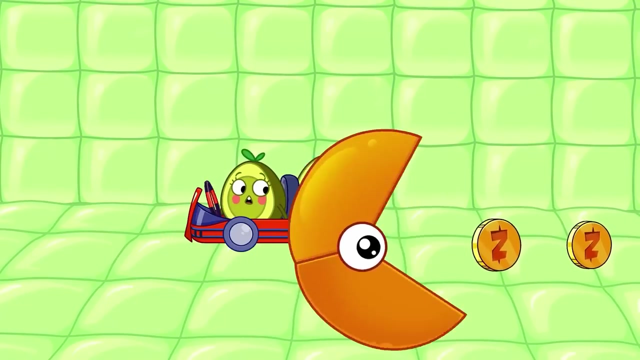 It's another power-up. Careful, Pit, The road is slippery, Penny. Pit needs help. Phew, He's safe. Thank you, Penny can't see. Uh-oh, I'm sorry. Now Pit and Penny are in the Munchman game. 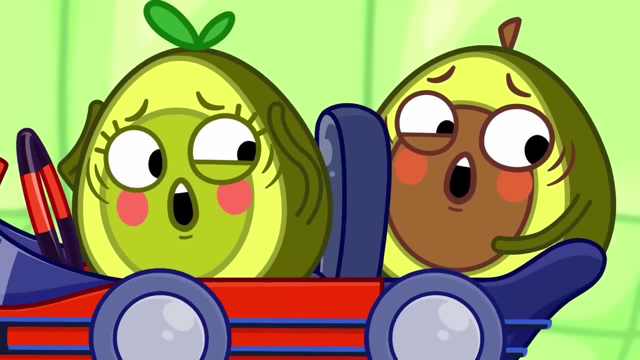 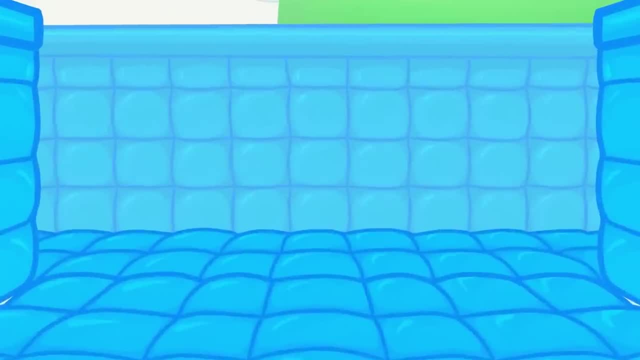 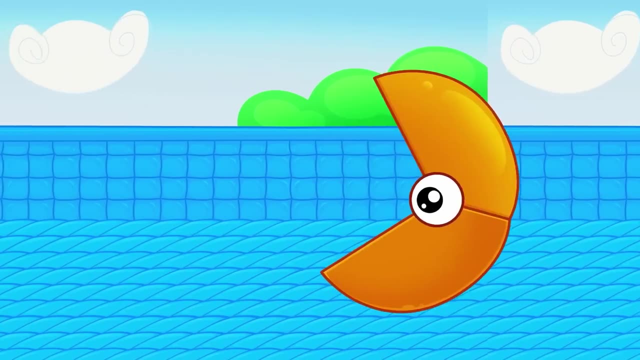 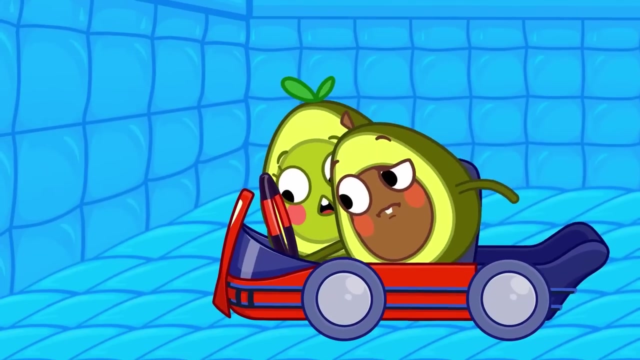 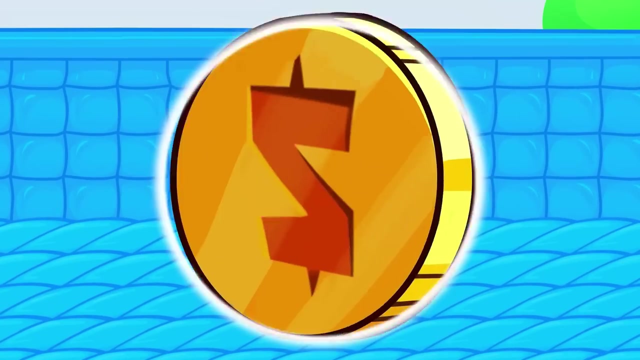 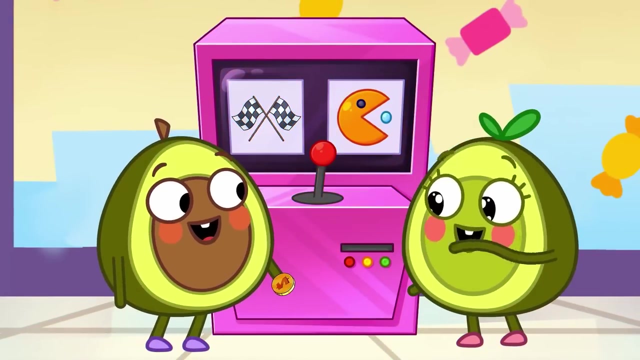 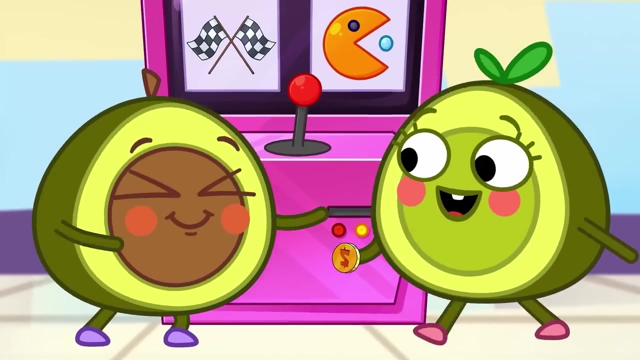 Munchman wants to eat them. Oh no, They're trapped. What should we do now? Jump out of it. Pit and Penny won the game And they're back to normal. Now they'll pick a game together. It's Officer Pumpkin. 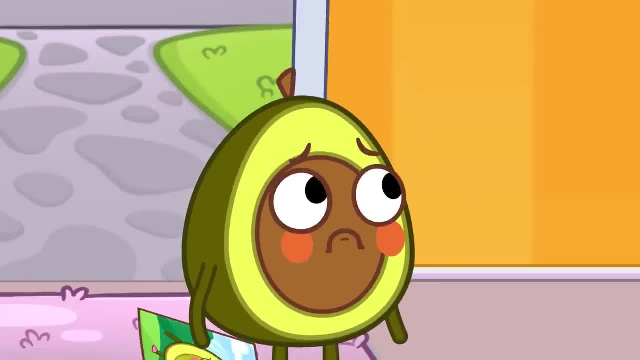 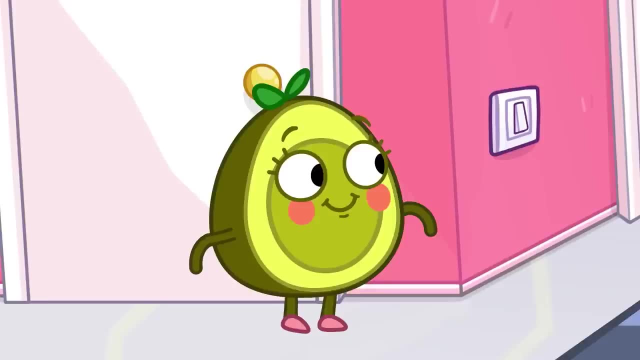 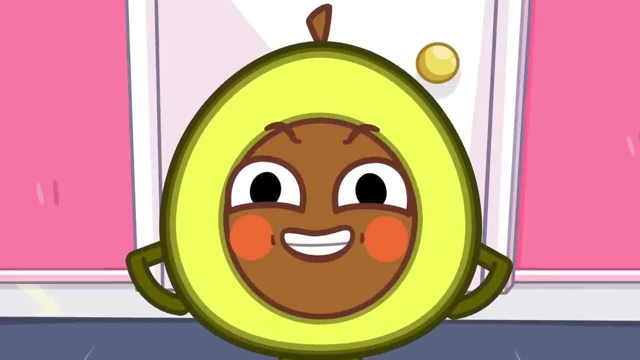 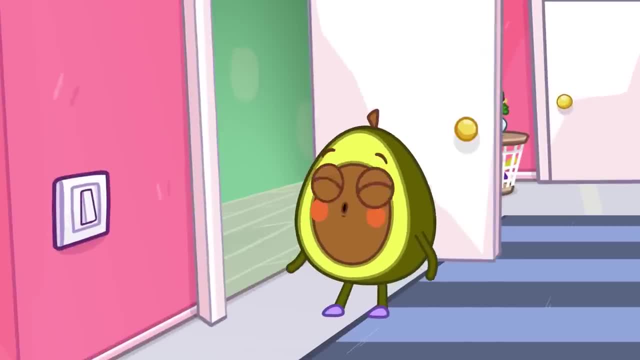 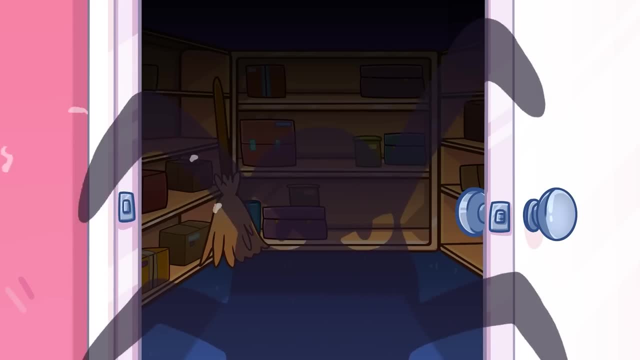 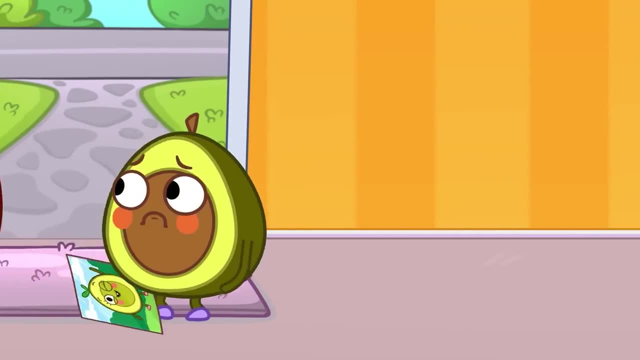 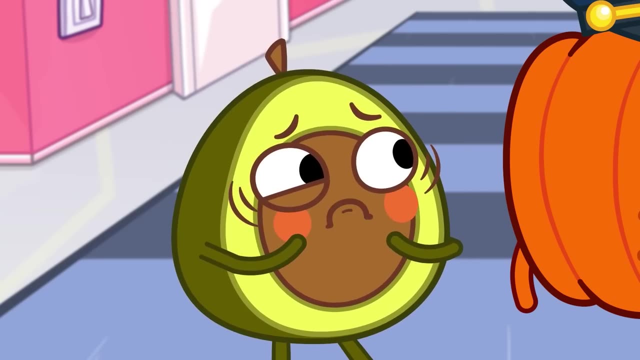 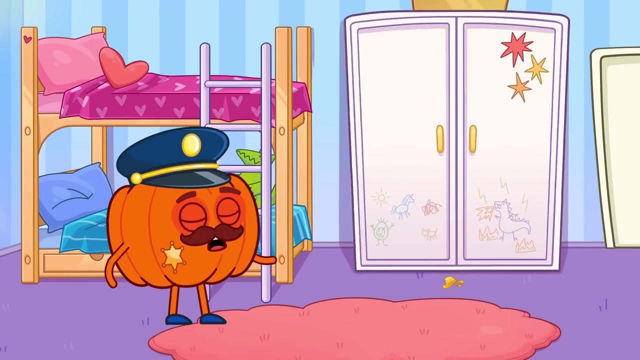 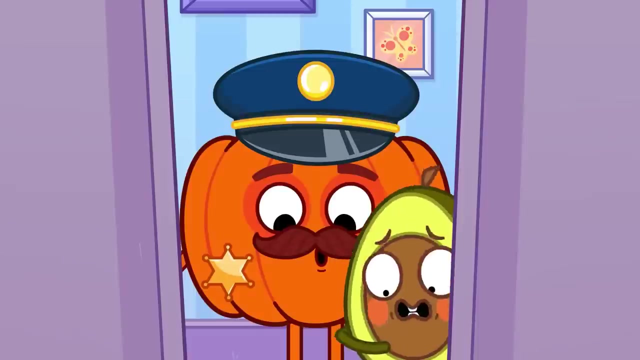 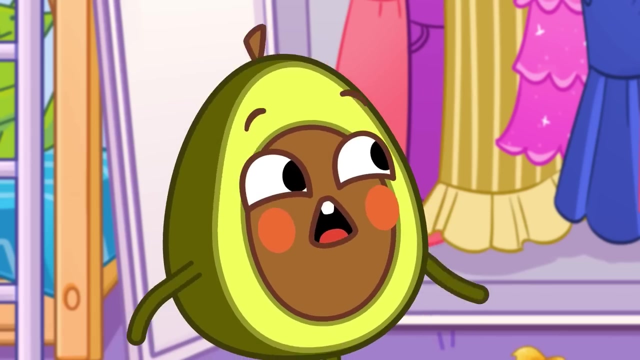 Officer Pumpkin will find her Penny. It's a monster. Hurry, Hurry. Check out that noise. It's coming from the wardrobe. Be careful, It's just a wind-up toy. Look, There are chips on the floor. 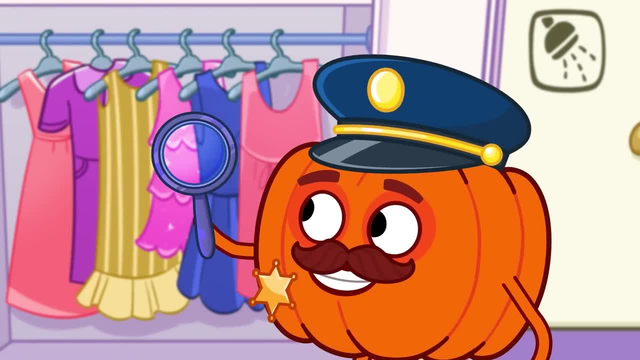 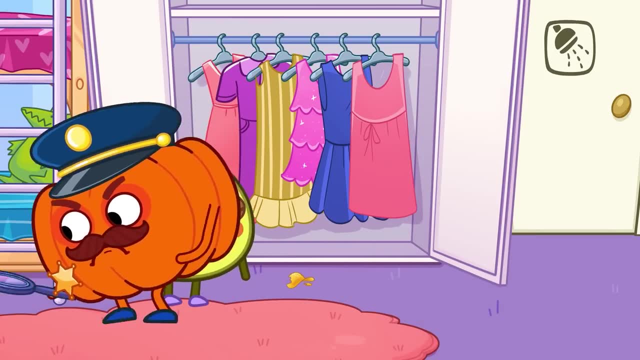 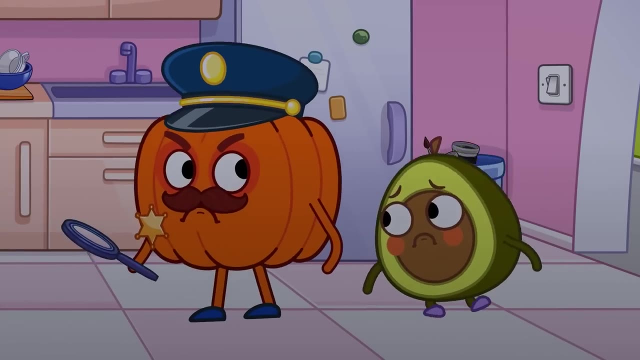 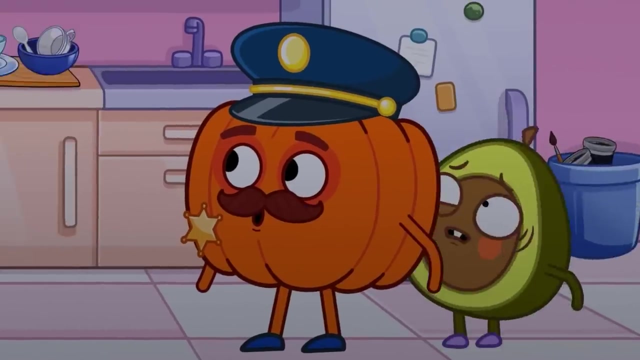 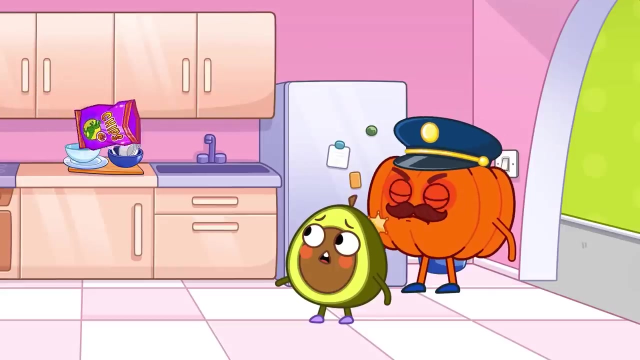 Maybe Penny left them. It could be a clue. Let's follow the trail. The trail leads to the kitchen. Is it the monster? A monster, A monster. No, Pit, It's an animal, It's an empty bag of chips. 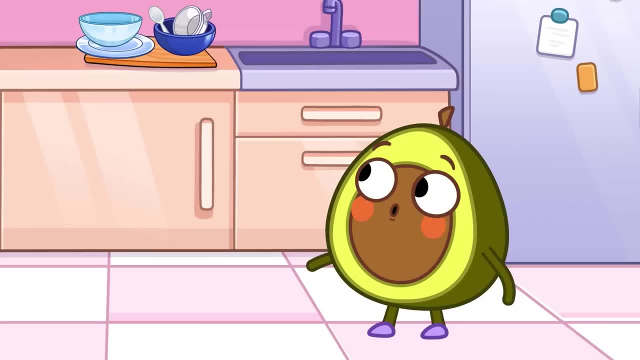 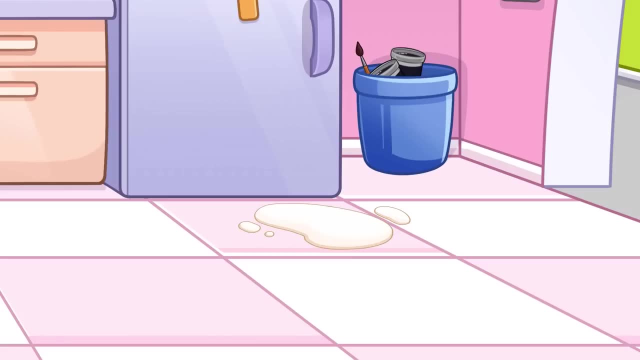 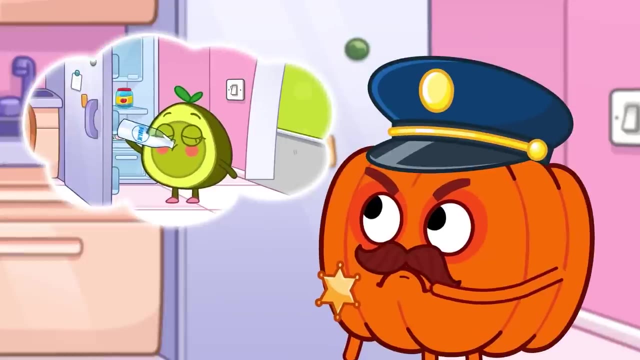 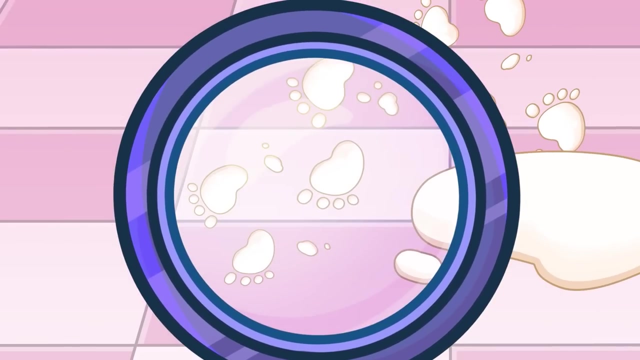 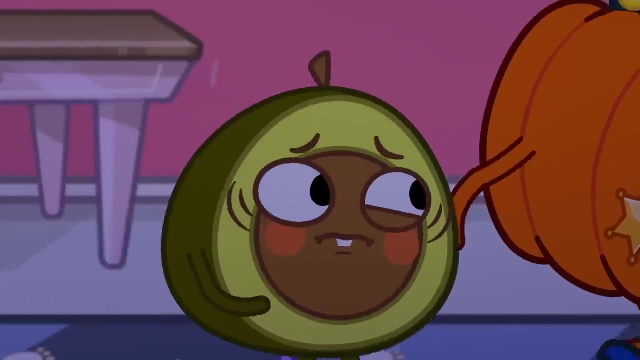 Someone left the window open, But where's Penny? There's milk on the floor. Maybe Penny drank some milk. Footprints- Another clue: Let's follow them, Don't be scared. Pit The footprints, stop. So where is Penny? 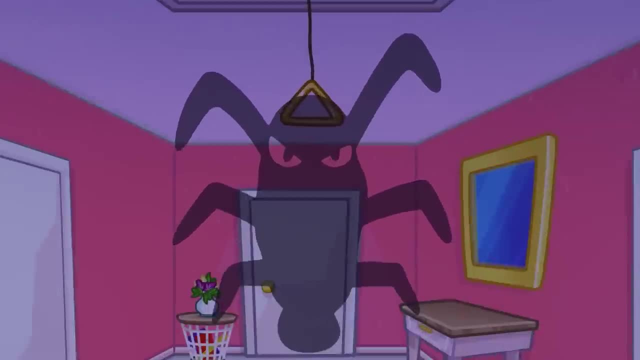 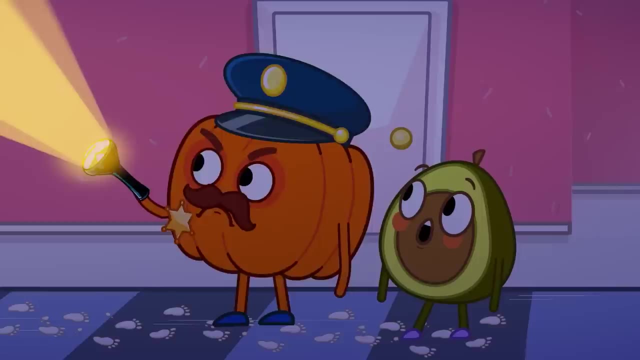 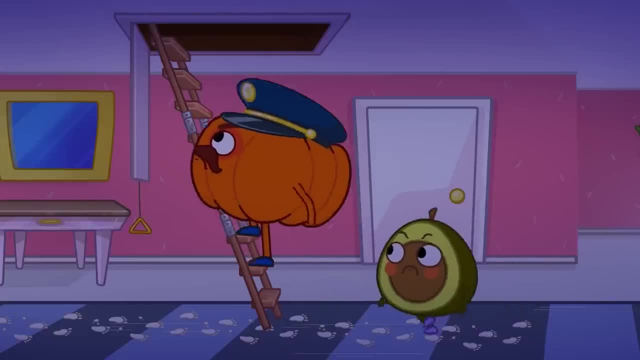 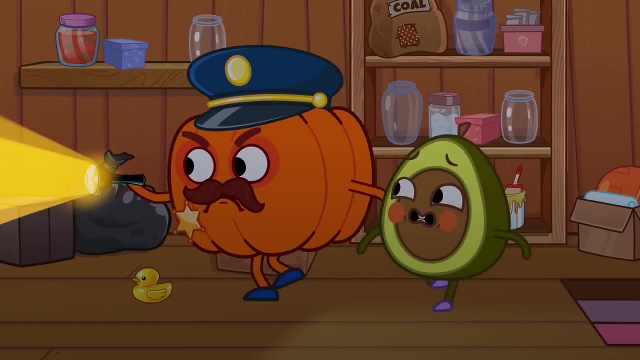 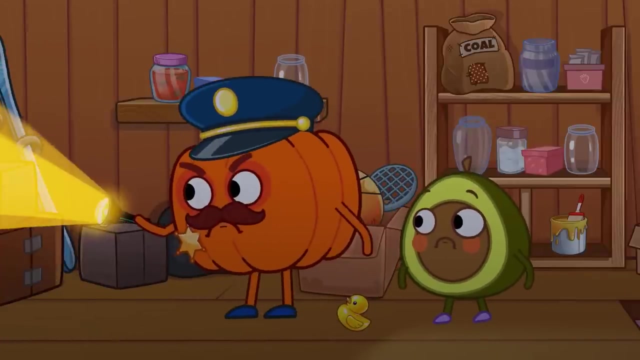 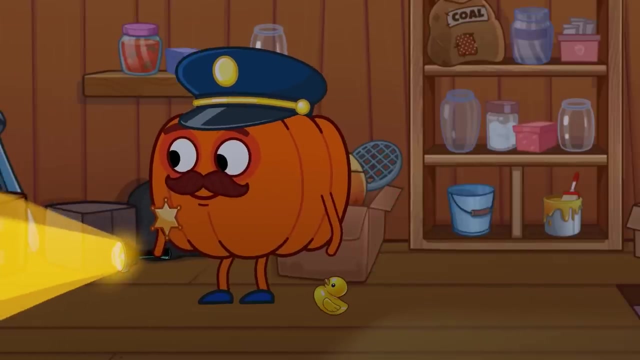 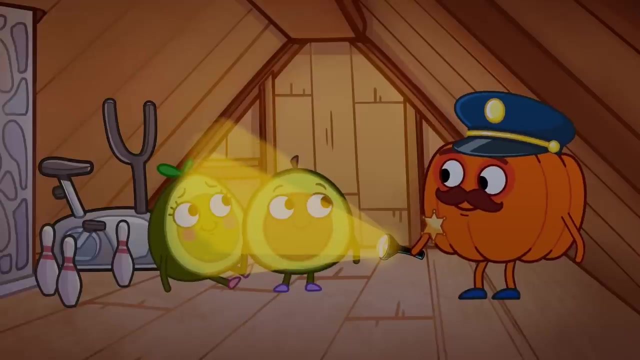 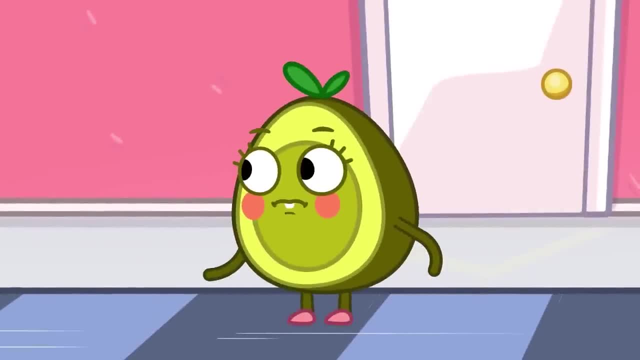 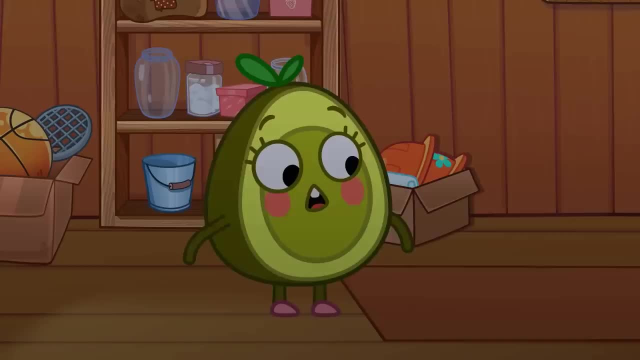 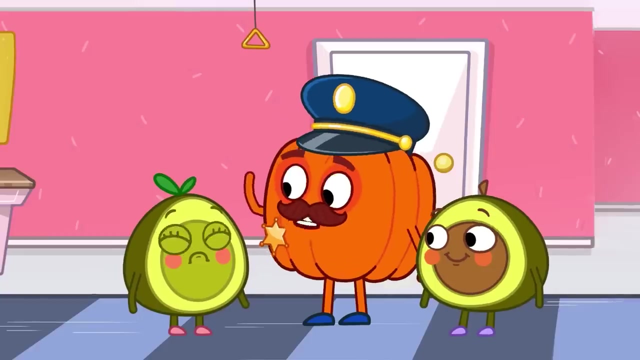 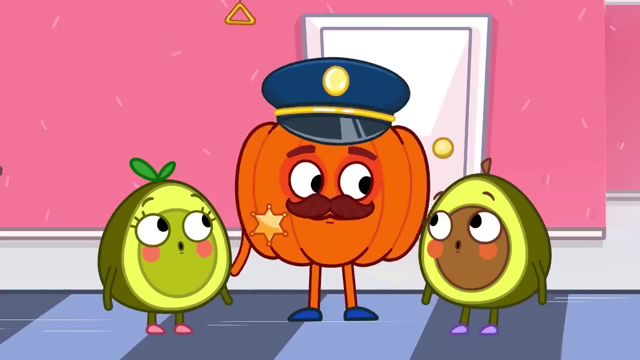 How did that happen? When Penny was looking for a place to hide, she snuck into the attic, But the door closed and got stuck. You can hide in places like the attic, basement or closet. They can be dangerous. Goodbye, little spider. 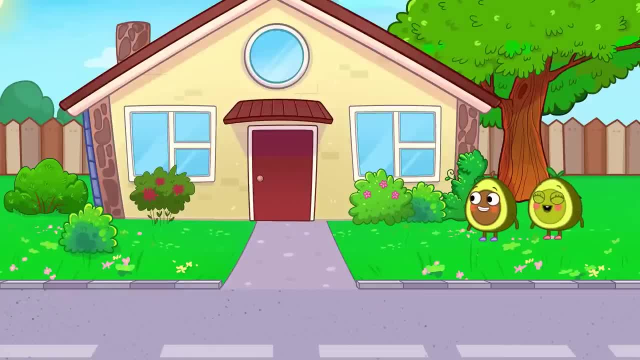 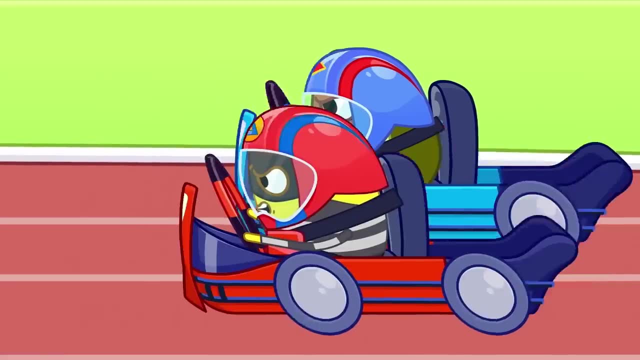 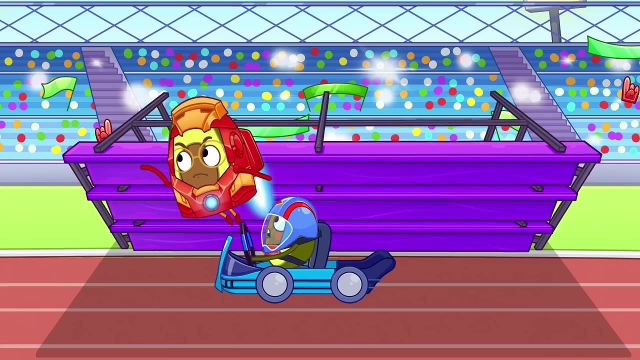 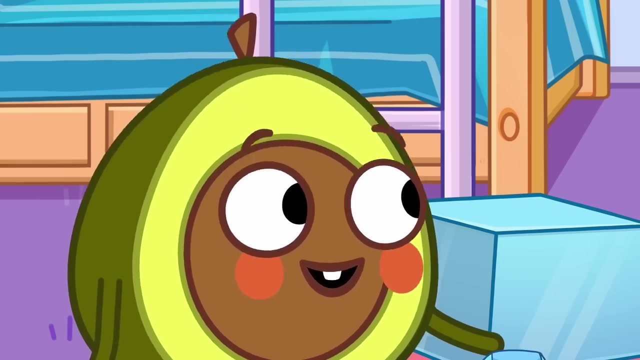 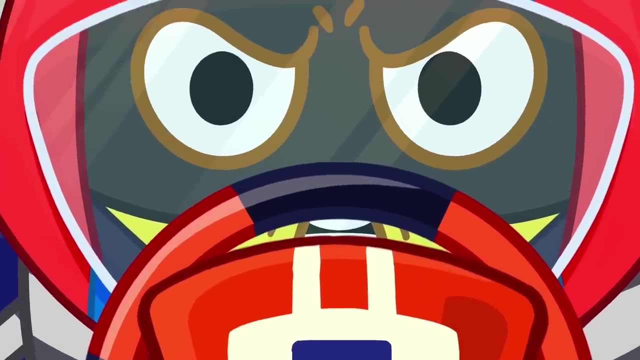 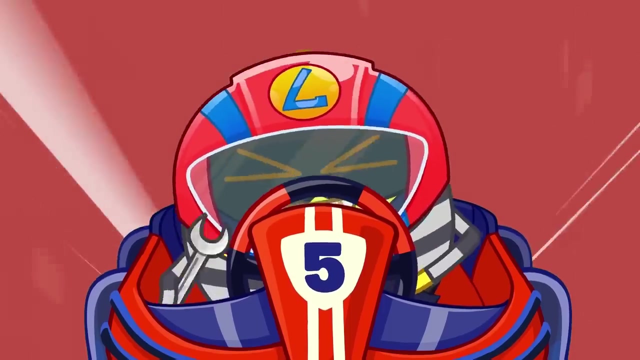 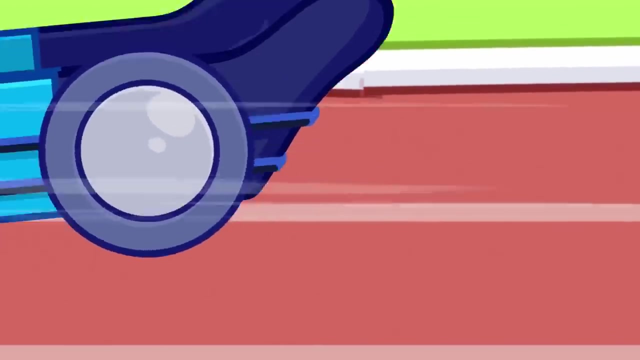 And goodbye, Officer Pumpkin. Thanks for your help. Pit is in a race And so is Mr Lemon. Watch out Pit. Super Daddy saved him. Go ahead, Pit. Pit takes the lead. Mr Lemon is cheating. The car's tire fell off. 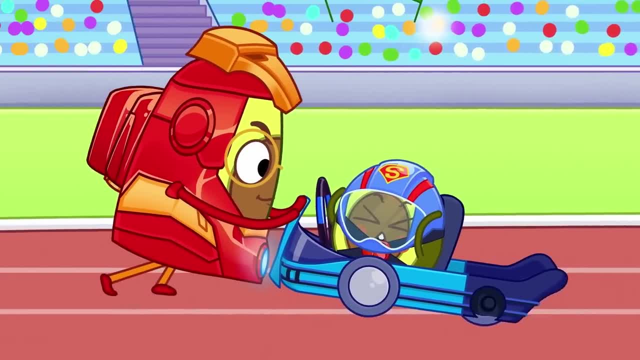 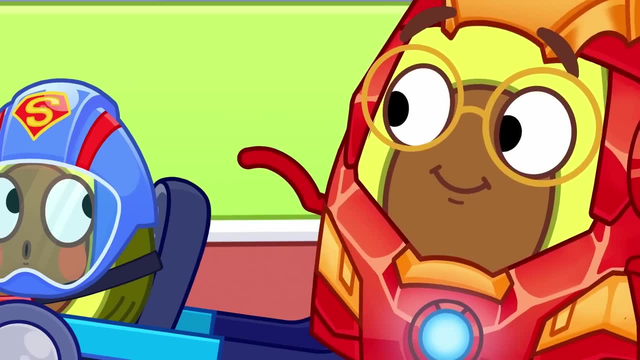 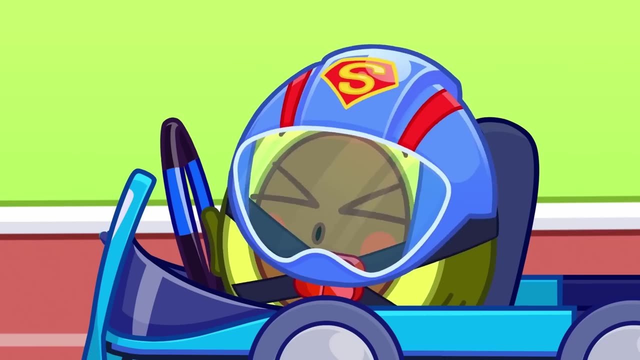 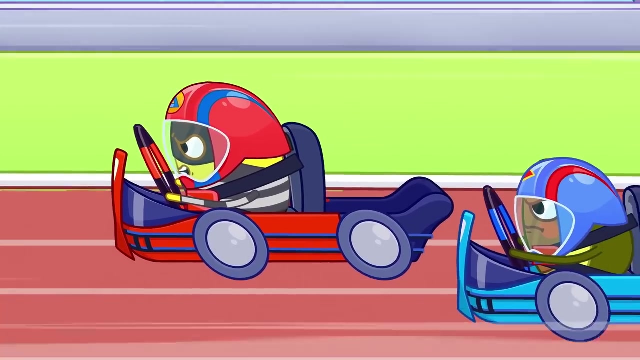 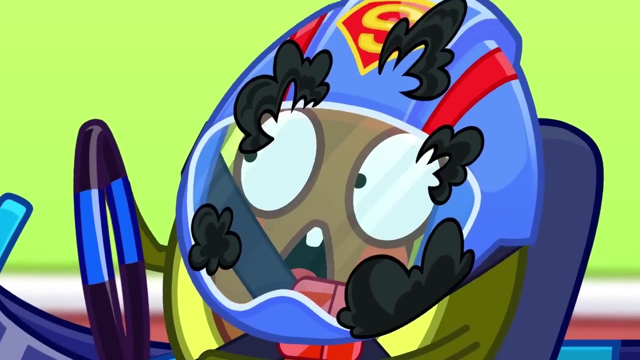 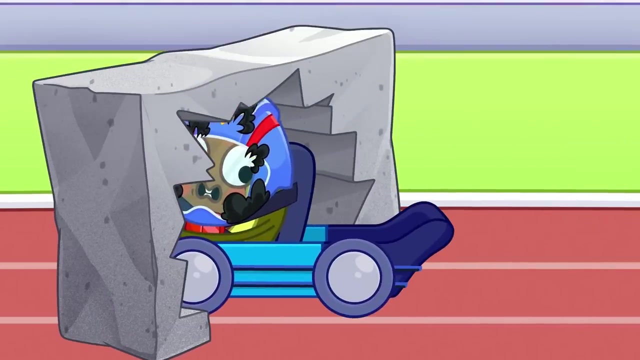 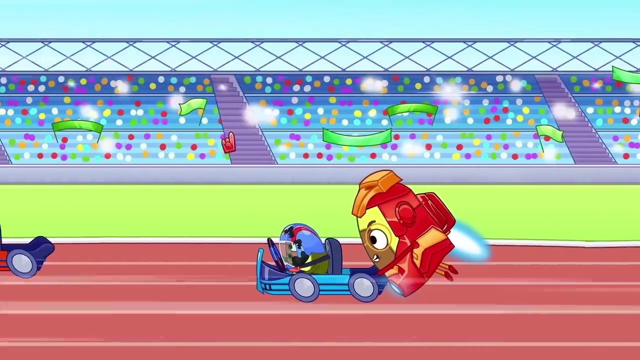 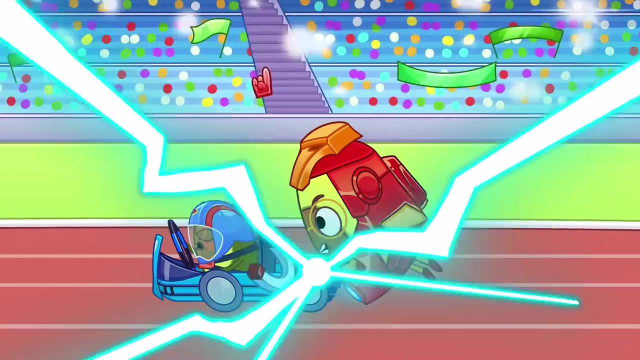 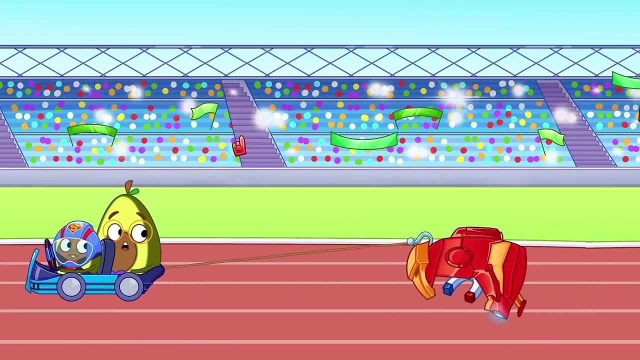 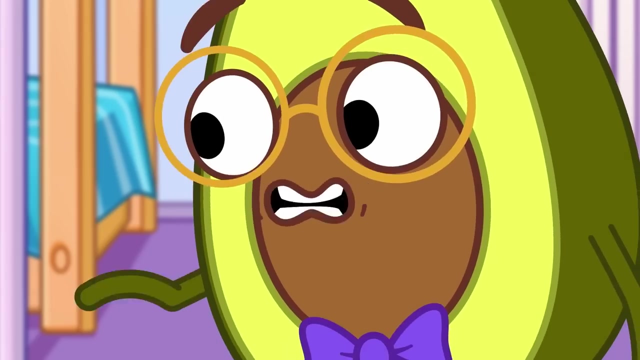 Super Daddy did it again. He'll fix that tire in no time. Pit's catching up. Oh Huh, Hurry, Super Daddy, Pit's stuck. Mr Lemon has more tricks. Come on, Pit Daddy's stepping on the toy. 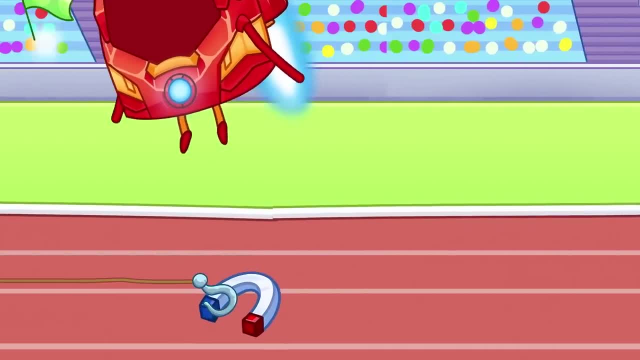 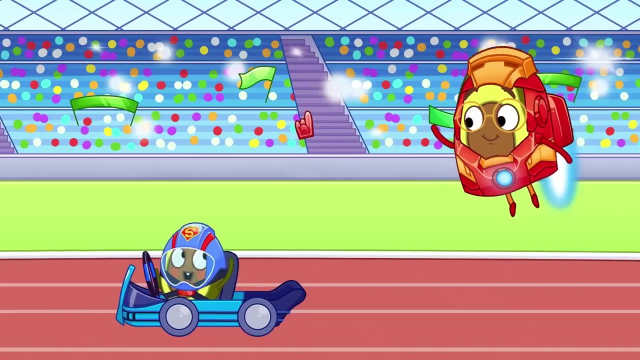 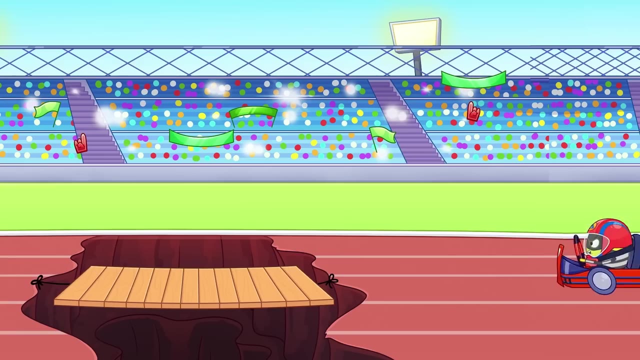 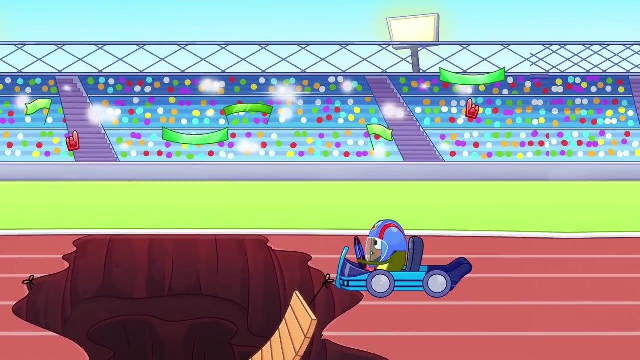 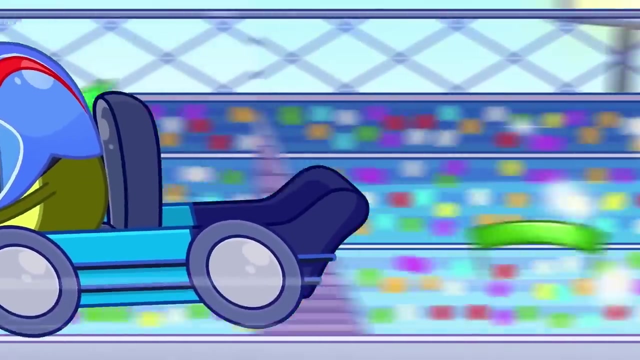 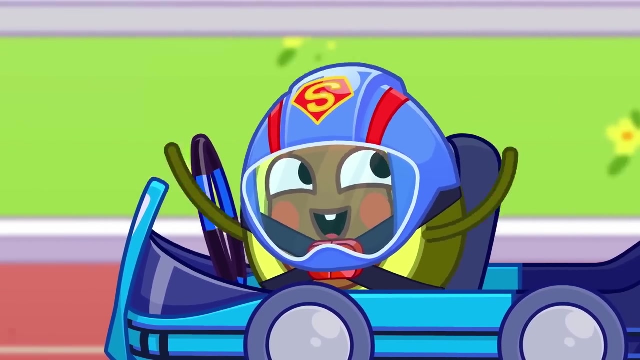 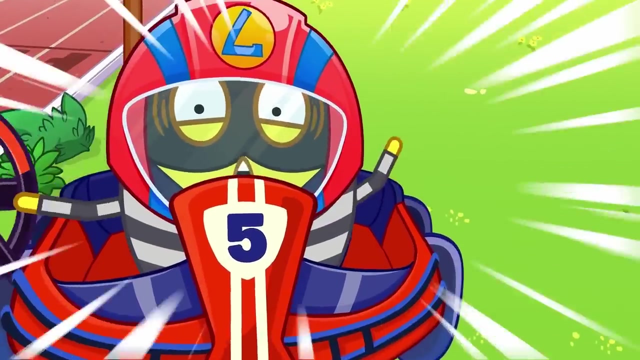 But how will Pit win Super Daddy's back to help? The bridge is broken. Super Daddy knows what to do. Pit wins the race. Mr Lemon's car is going to crash. Super Daddy to the rescue. Thank you and sorry for everything. 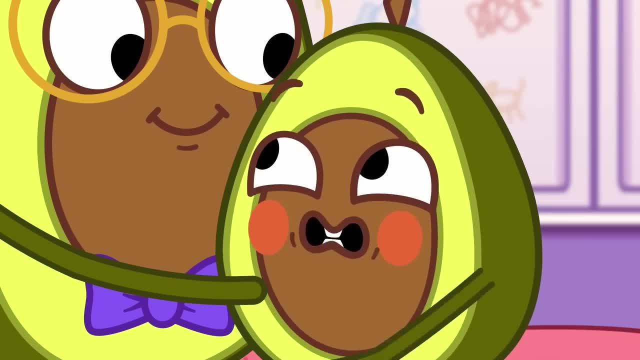 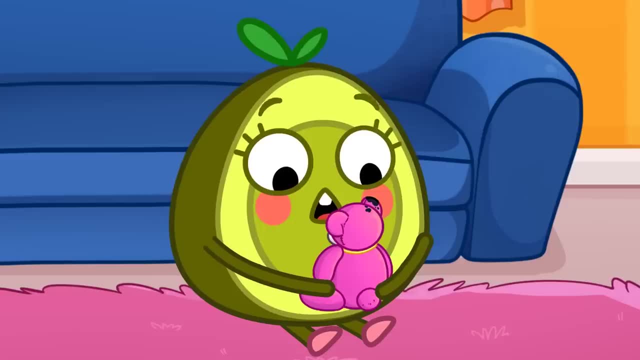 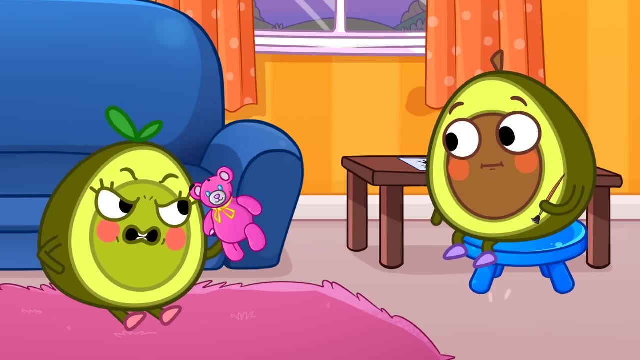 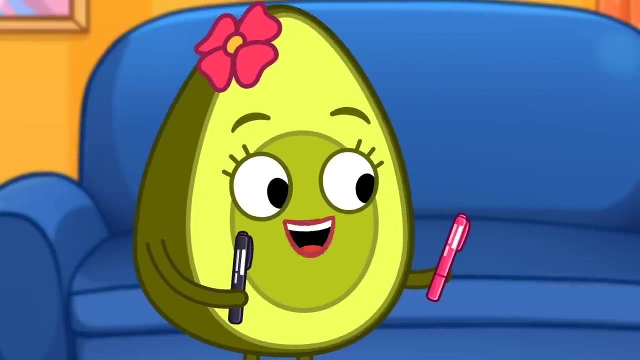 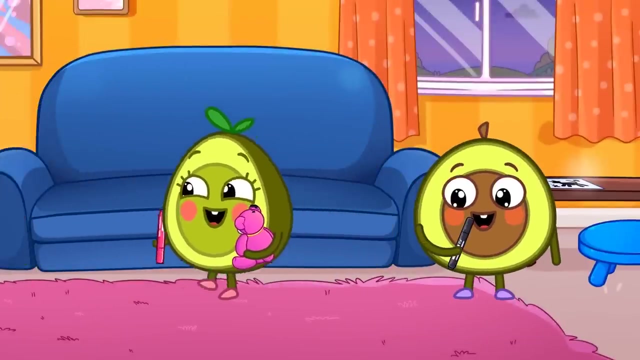 Pit has something to say. My daddy's a superman. What's that on your pink bear, Penny? It's black paint, Pit, please be more careful. Mommy gives Pit and Penny magical pens, But be careful with those. It's a pink bear. 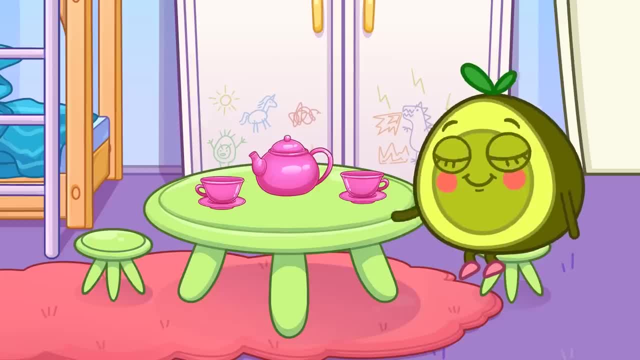 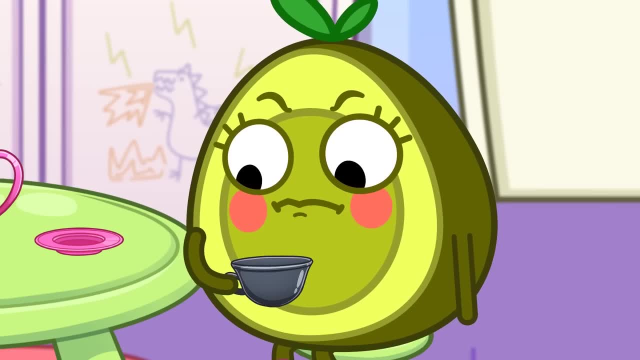 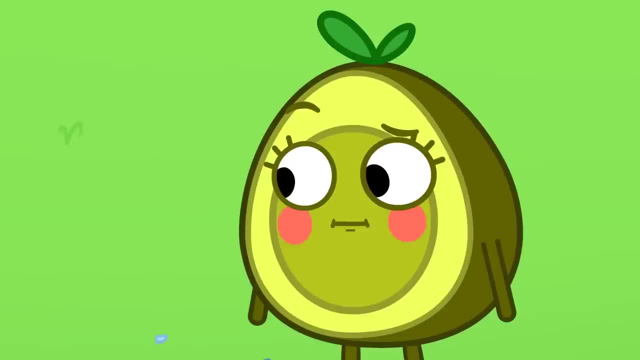 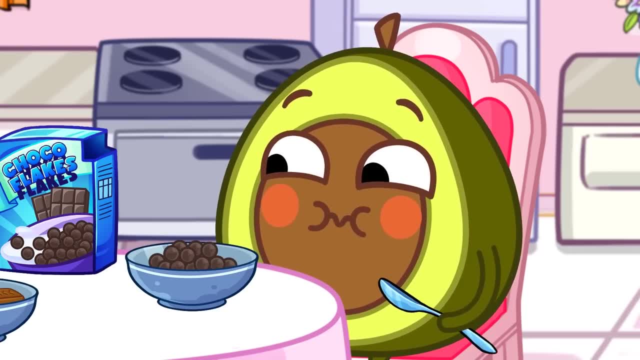 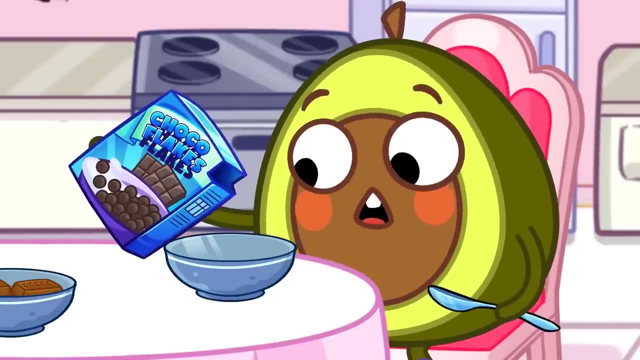 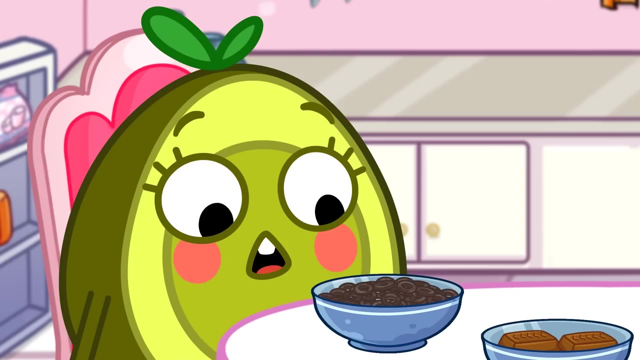 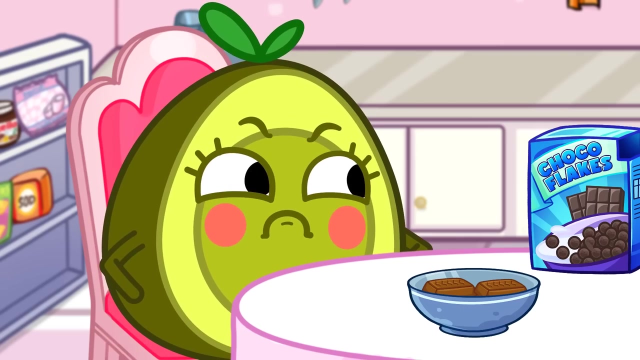 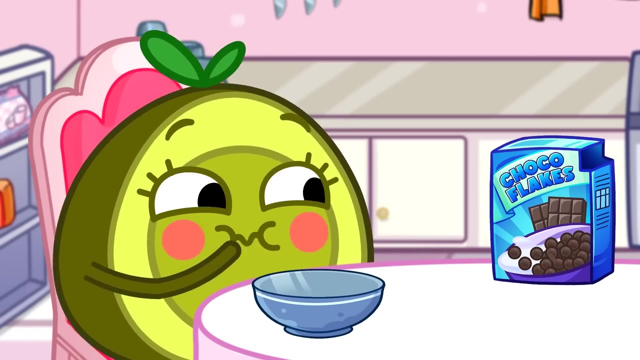 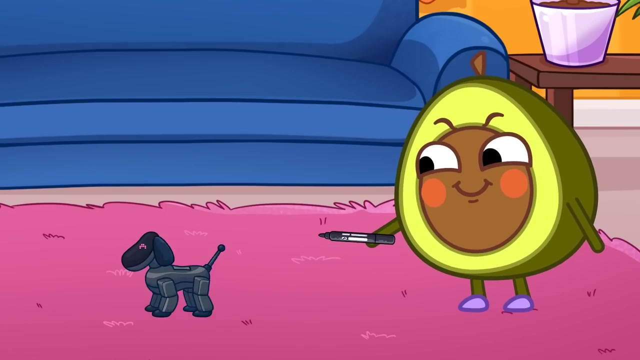 It's breakfast time. At least you two are getting along. Oh, hit Now. Penny won't eat it, But she will eat the pink cookies. This toy is not black or pink. It's blue. Now it's black And now it's pink. 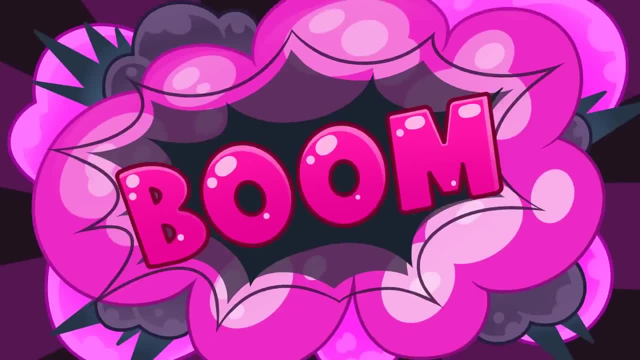 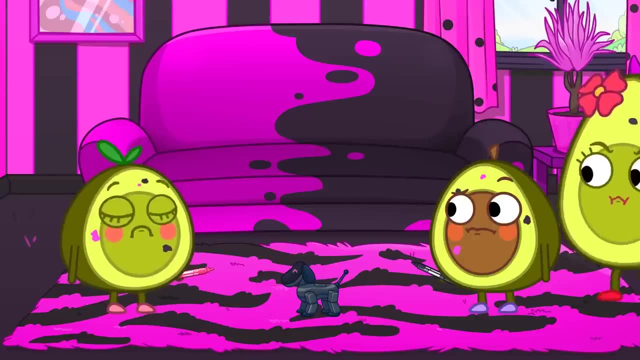 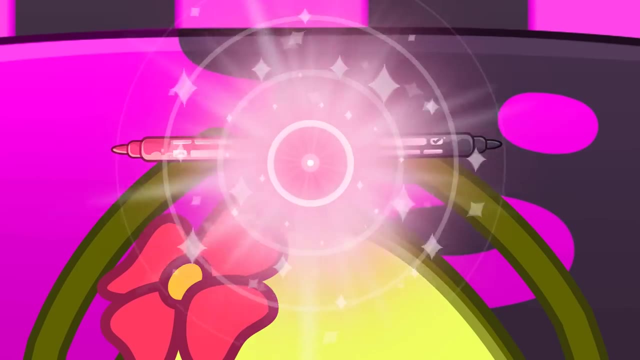 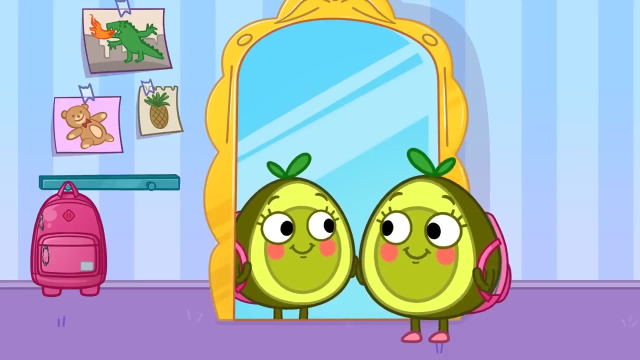 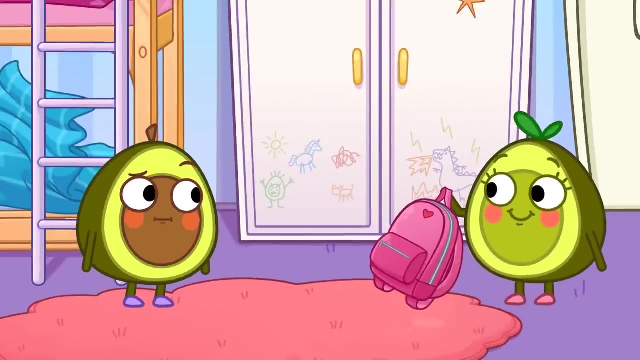 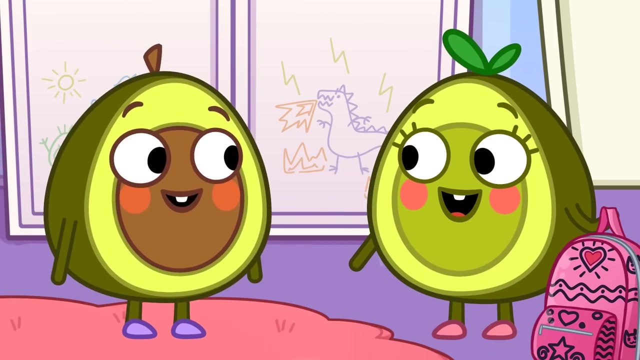 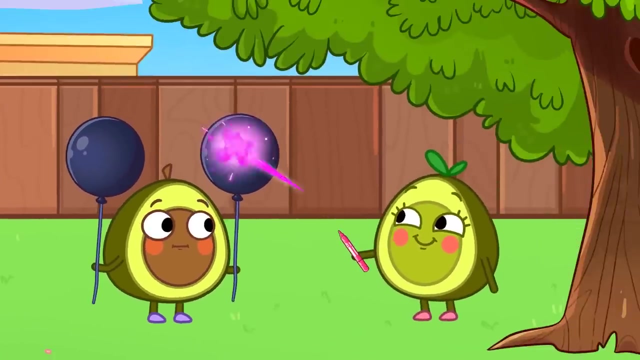 See, Be careful. What will Mommy think? Give Mommy your pens. Penny has a pink backpack. Maybe a little black would make it better. How cool. Hit has two black balloons. Why not add some pink? See, Black and pink are perfect together. 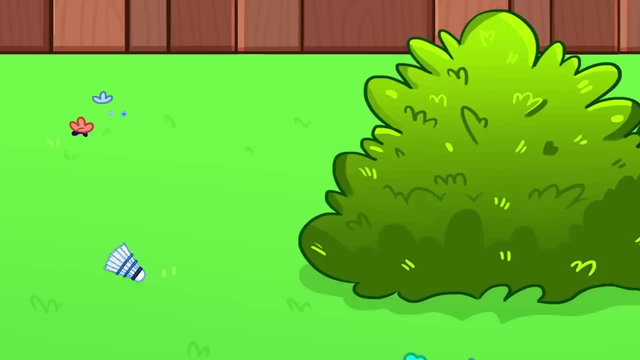 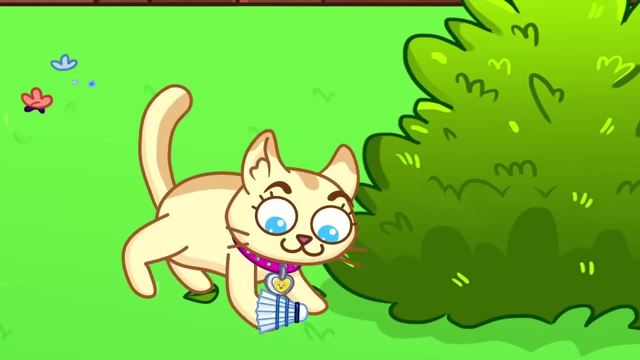 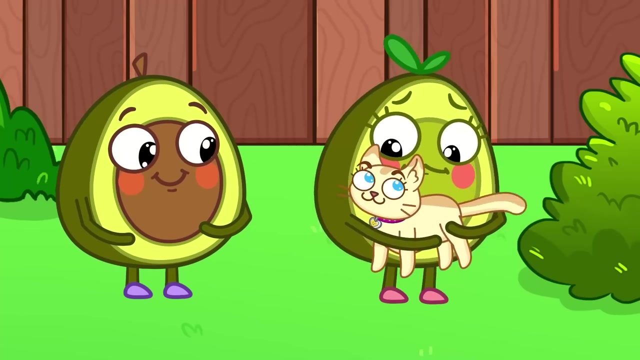 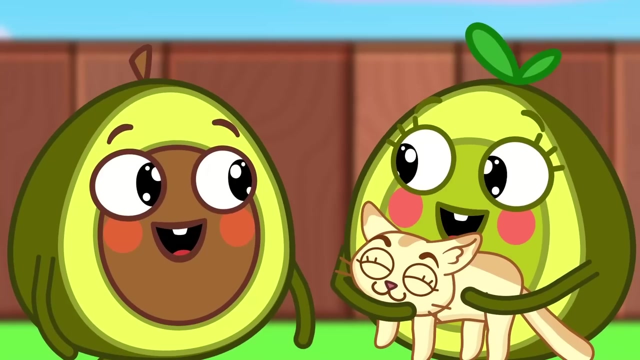 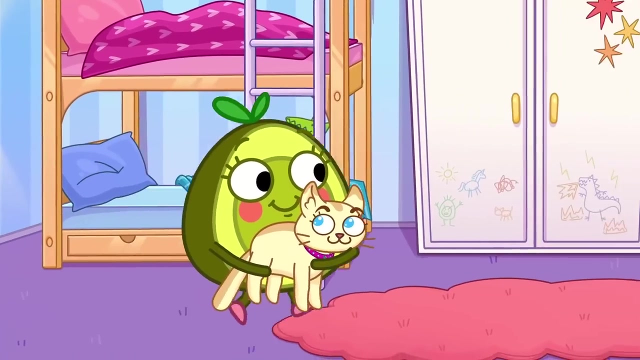 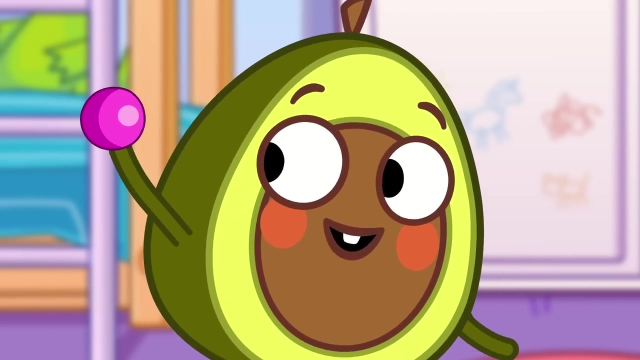 Hit and Penny are playing badminton. Oh look, It's a cute little kitten. Be gentle Penny, Let's take him home. The kids have taken the kitten to their room. Pit wants to play fetch with the kitties. 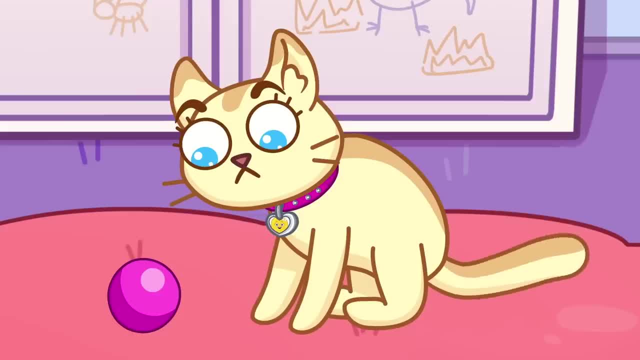 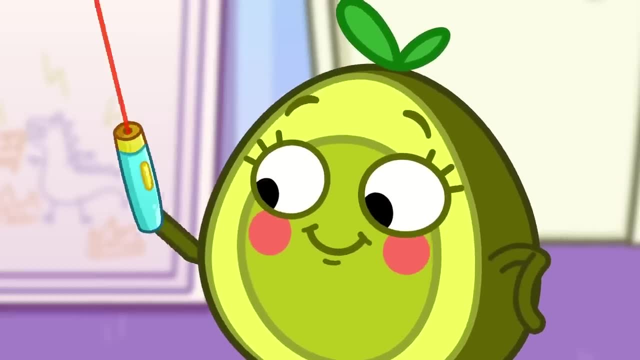 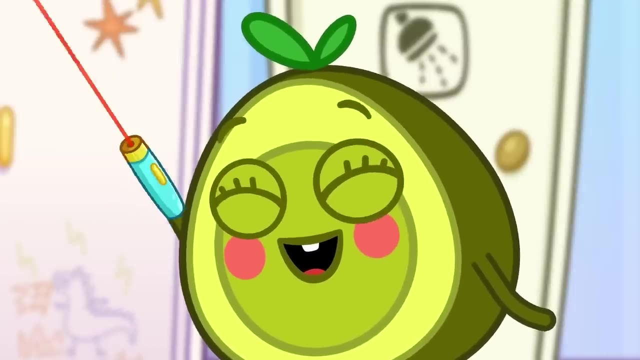 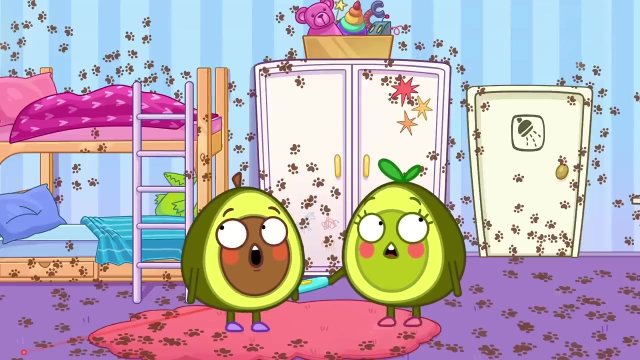 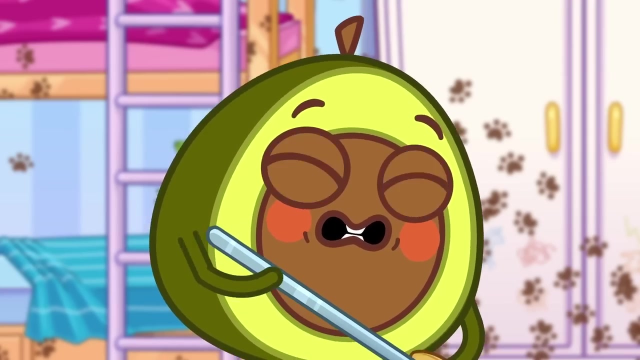 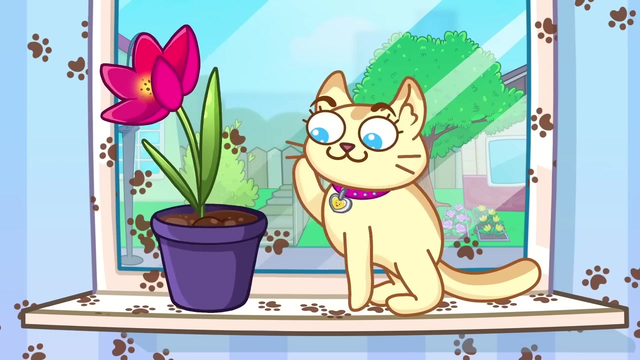 But most kittens don't play fetch. Kittens do like to chase light. right, Penny? Oh no, There are paw prints all over the room. You better clean it up before Mommy sees it. What's that kitten? up to now, It's going to knock over the flower pot. 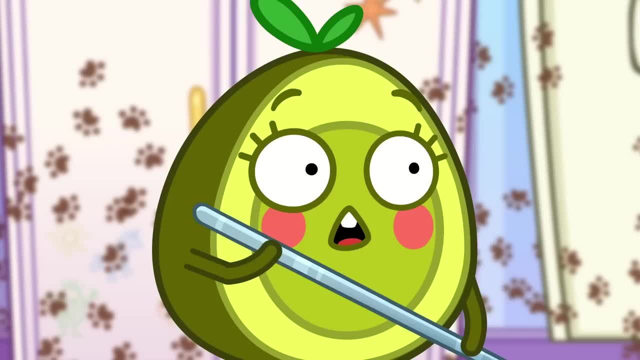 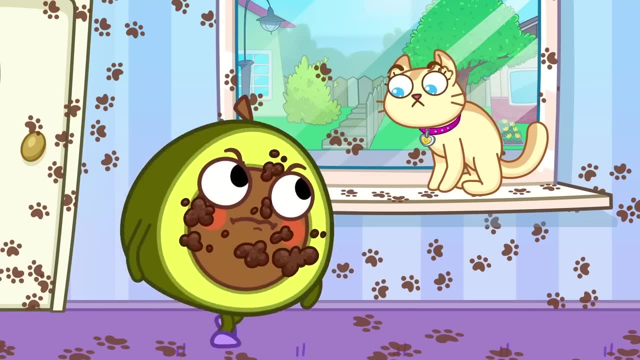 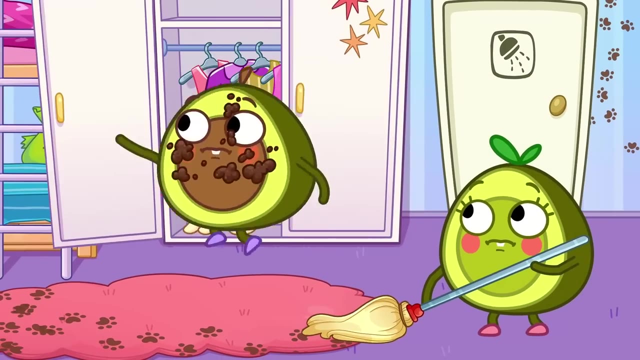 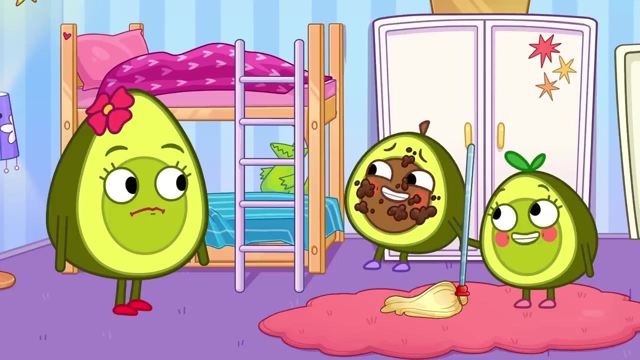 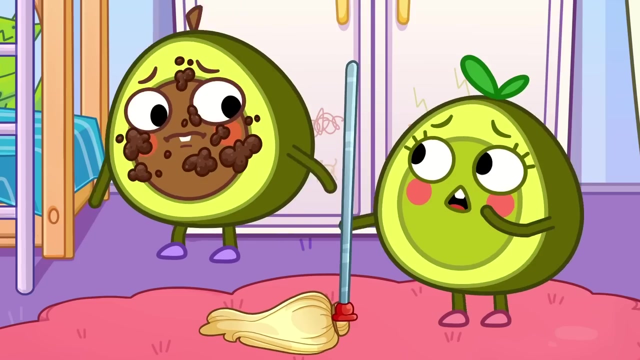 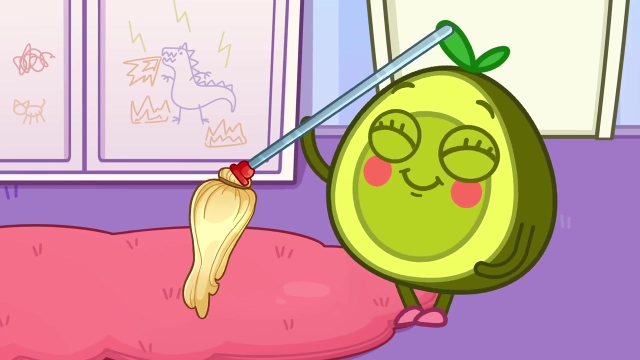 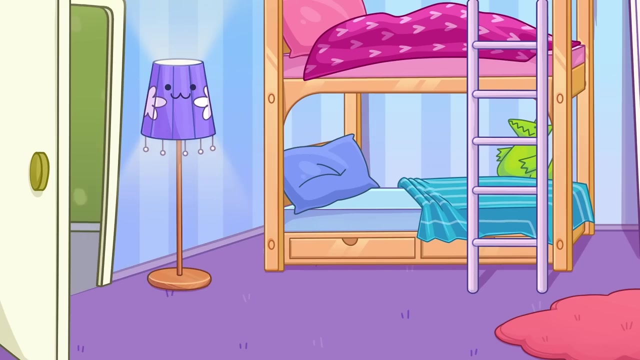 Oh no, What's happened, kids? Pit wants to hide the kitten. Here comes Mommy And she sees the broken pot. I'm sorry, Mom, I've broken it. Oh, I'll clean it. Pit, you can't hide that kitten forever. 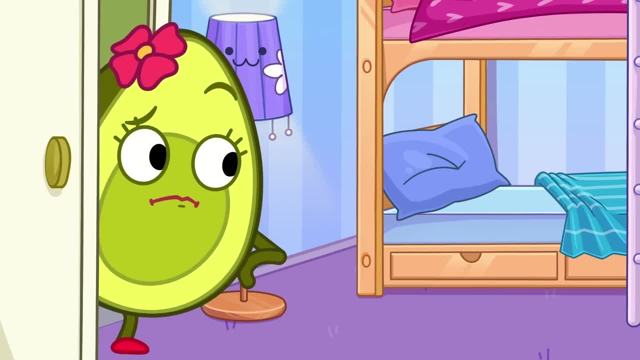 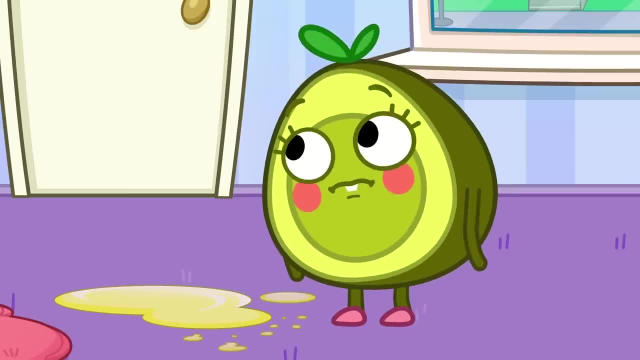 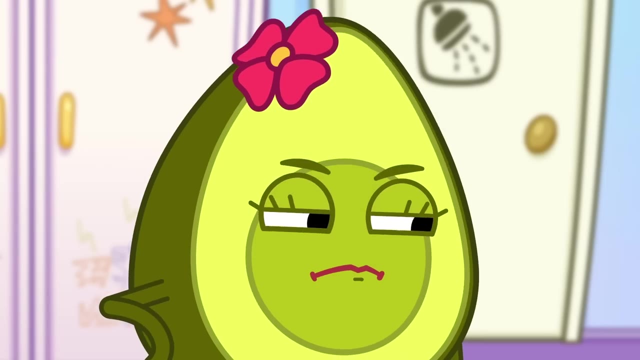 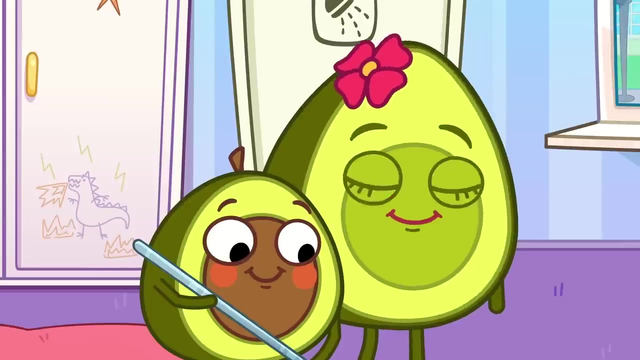 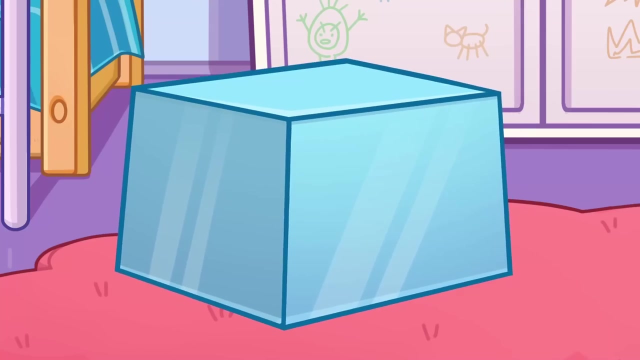 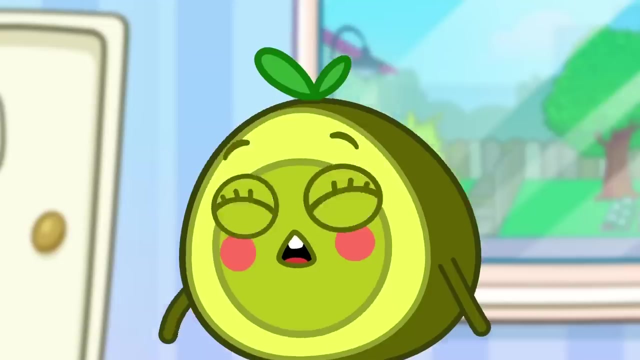 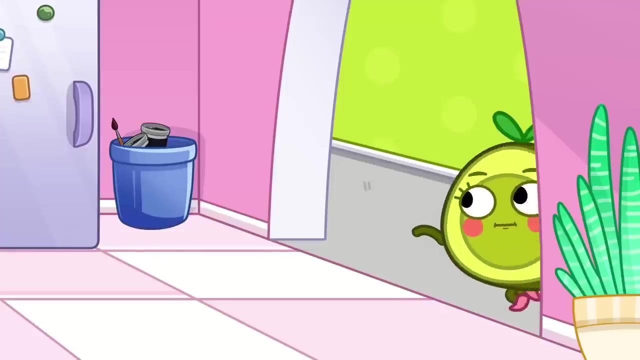 Uh-oh, The kitten got scared and left a mess on the floor. Oh, Do you have something to tell Mommy? It was me. Pit will clean it up. Thank you, Pit. Kittens need food. Penny will find something to feed her. 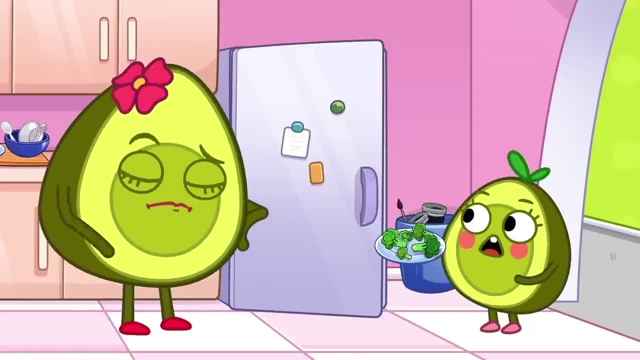 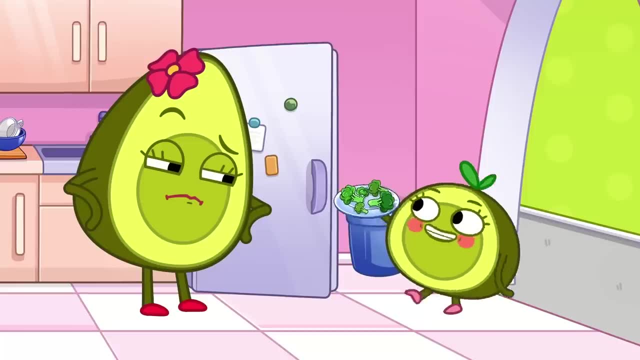 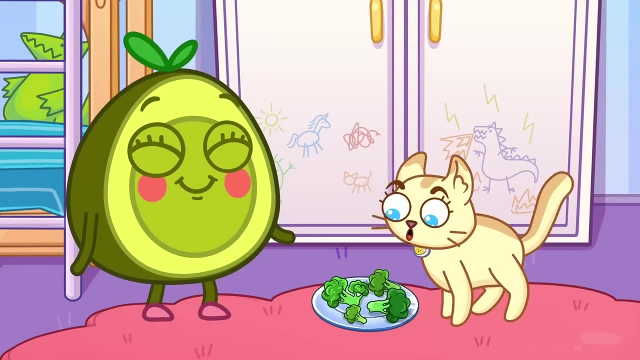 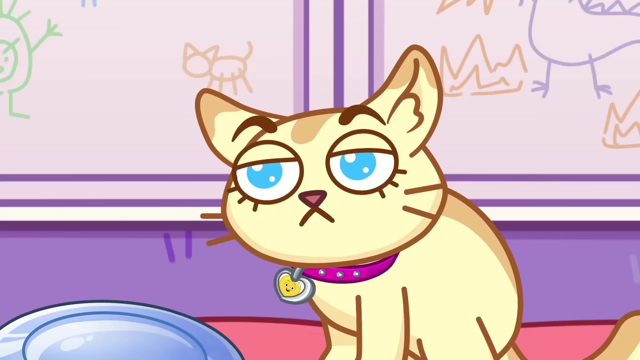 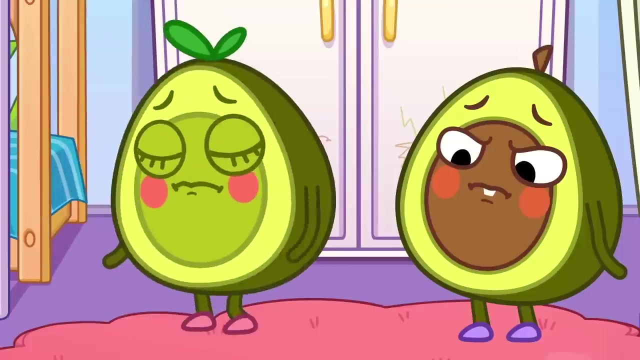 Broccoli? I don't know, Penny. Hmm, I love vegetables. Do kittens love vegetables? Meow, Meow, Meow. Nope, they don't Aw. The kitten needs a nap. Taking care of a pet is a lot of work. 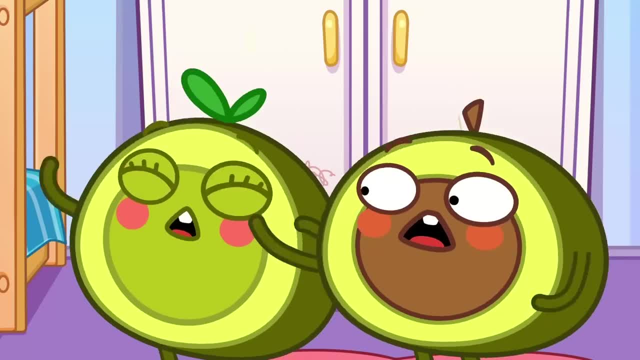 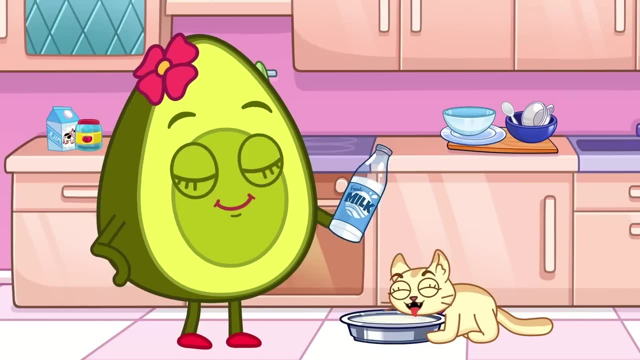 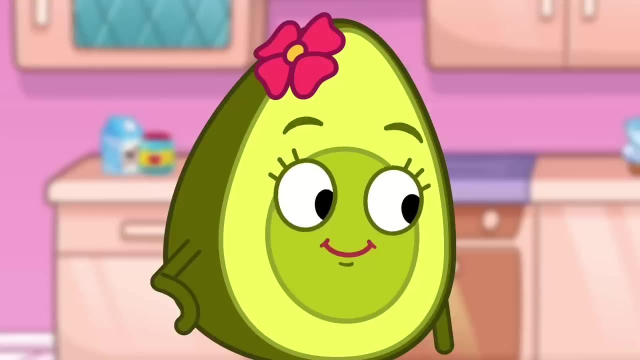 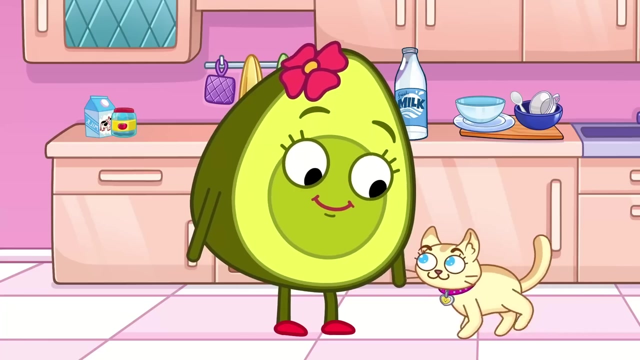 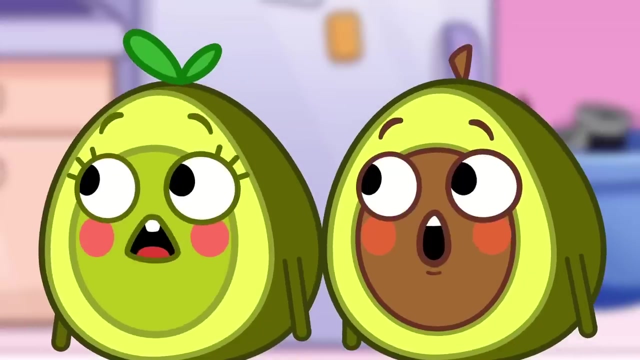 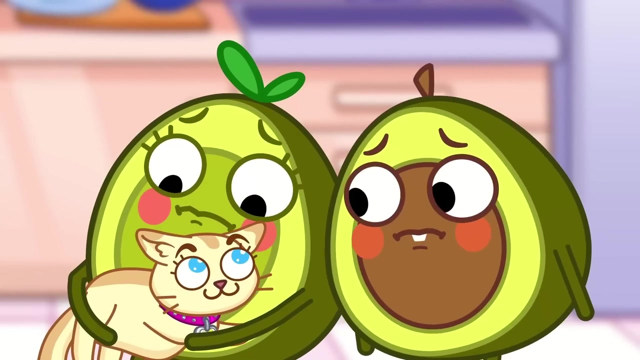 Where did the kitten go? There she is. Mommy is giving her milk. A kitten is not a toy. It needs a lot of care. Mommy knows what to do. It needs to be returned to its owner. Someone probably misses the kitten very much. 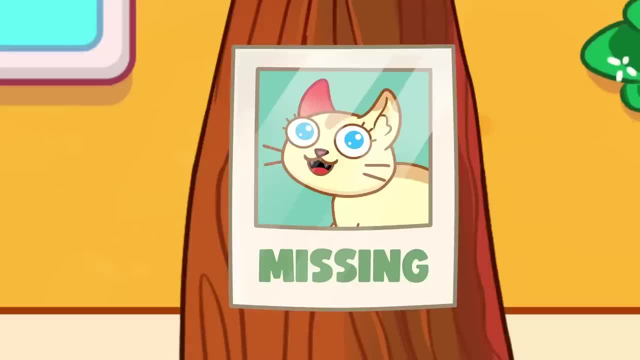 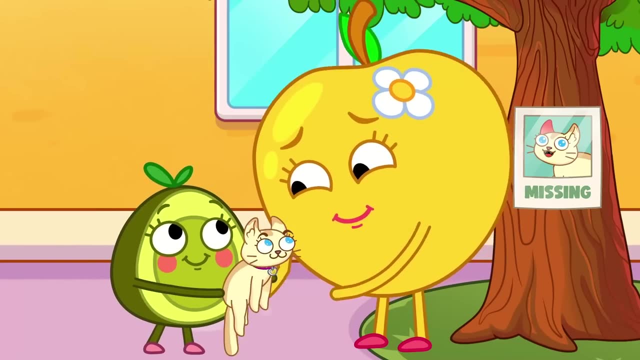 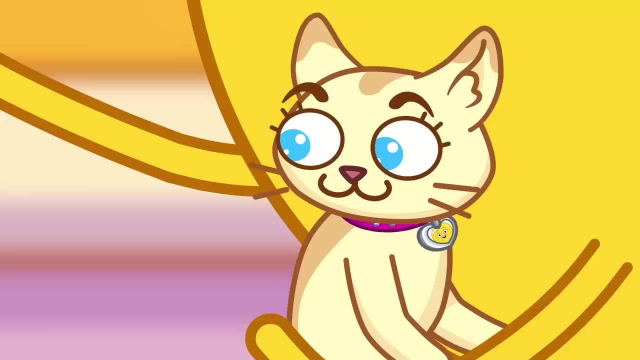 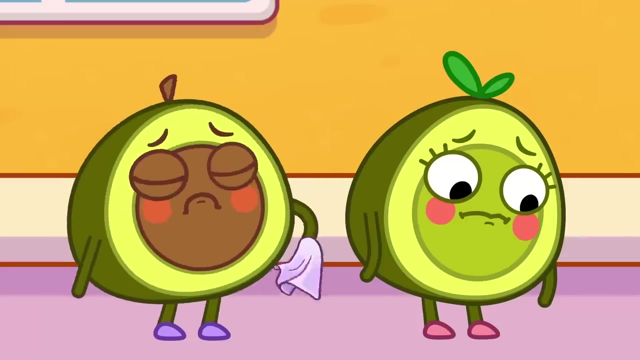 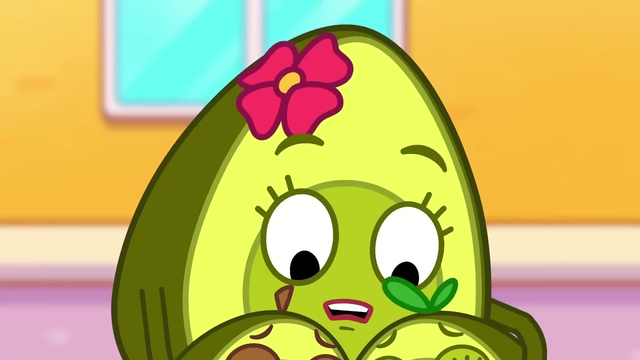 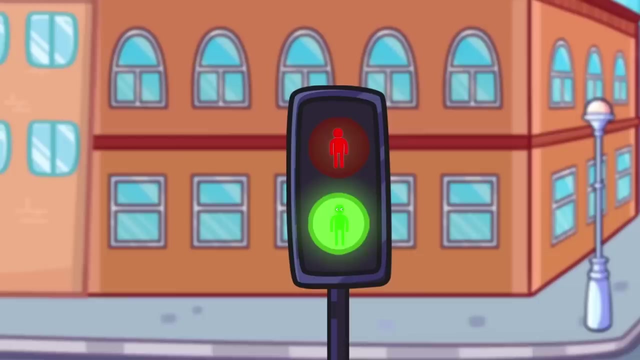 Miss Apple is sad and looking for her lost kitten. She's so happy to find her kitten again. See, Pit and Penny, You did the right thing. Well done kids. Pit and Penny are out for a walk, But they're not paying attention. 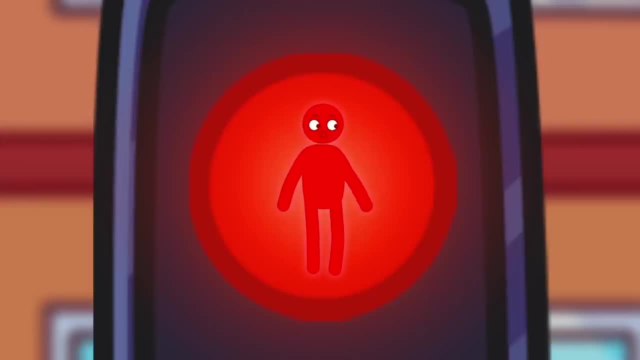 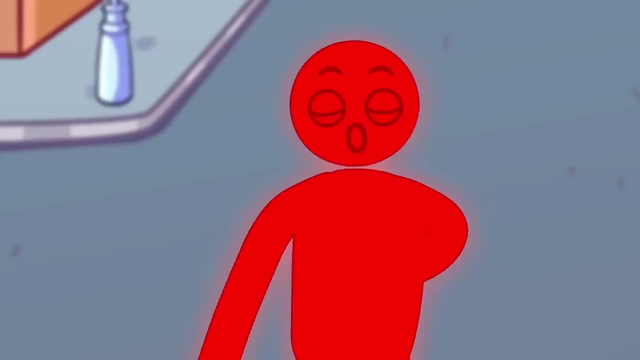 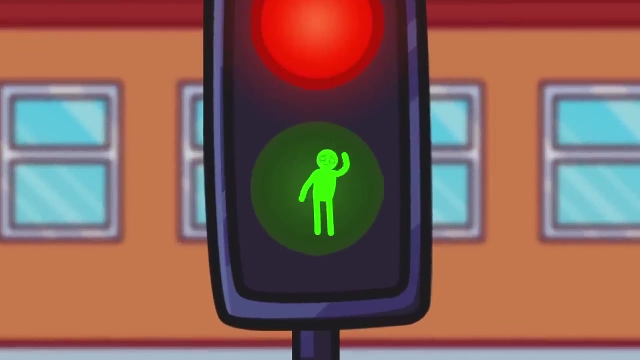 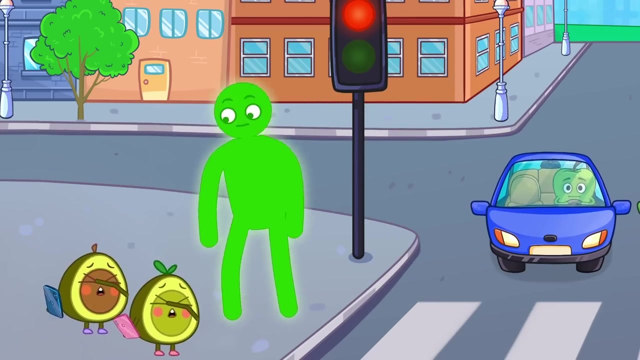 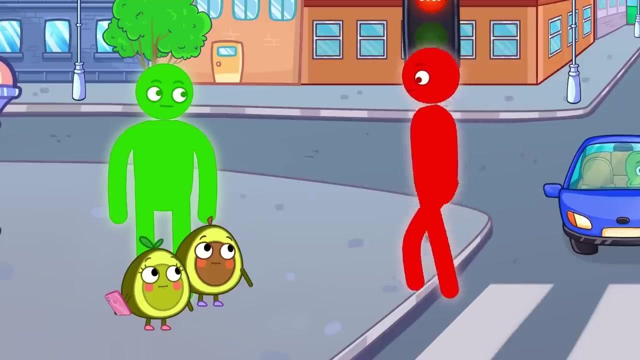 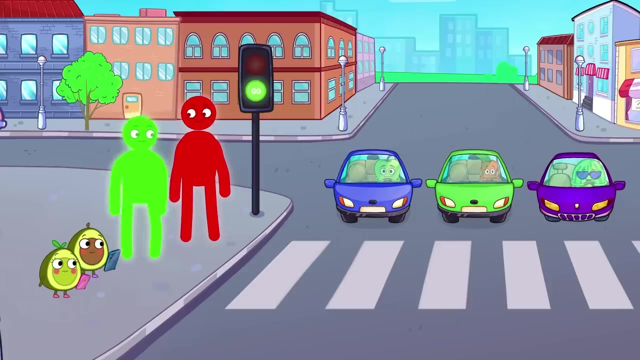 Oh no, The light changed to red. Someone needs to help Pit and Penny. It's okay, You're safe. Pit and Penny, Never use your phone while crossing the road. Don't cross the street when the light is red. When the light turns red, 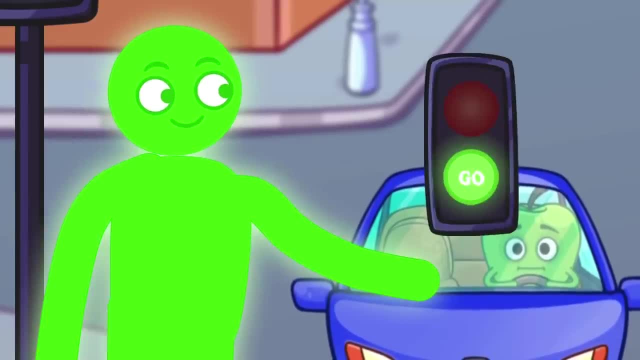 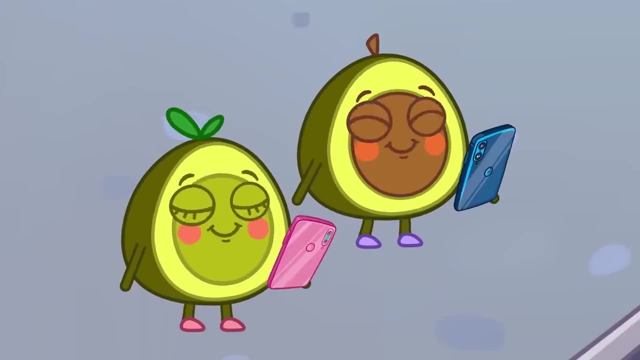 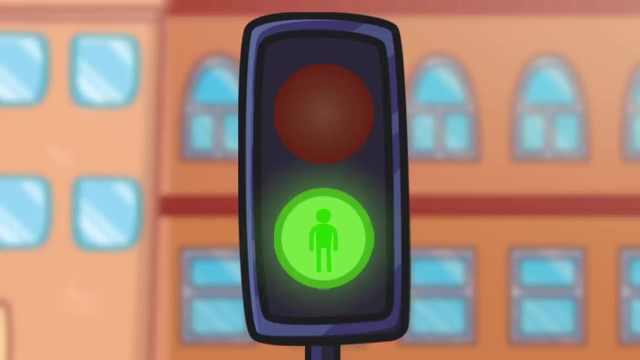 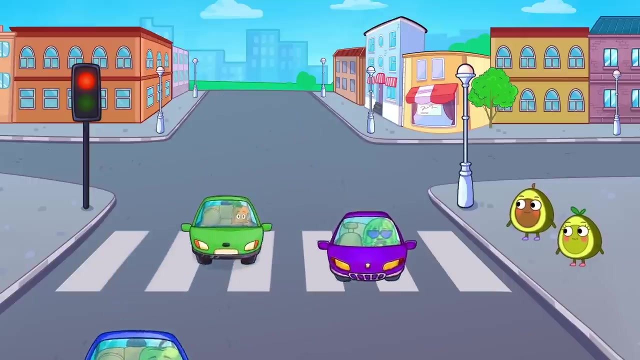 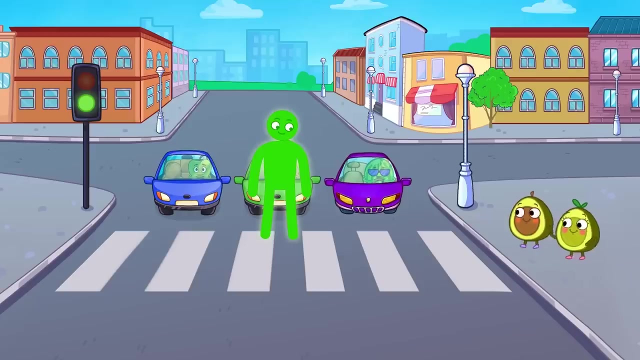 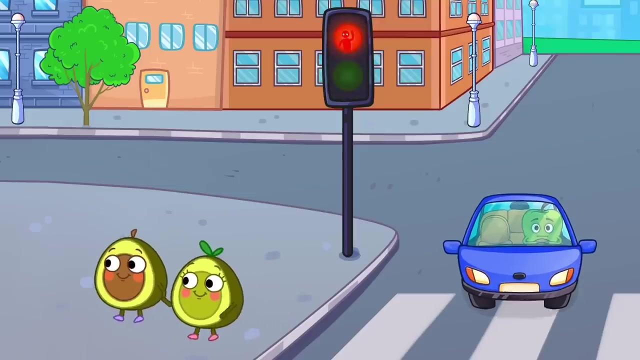 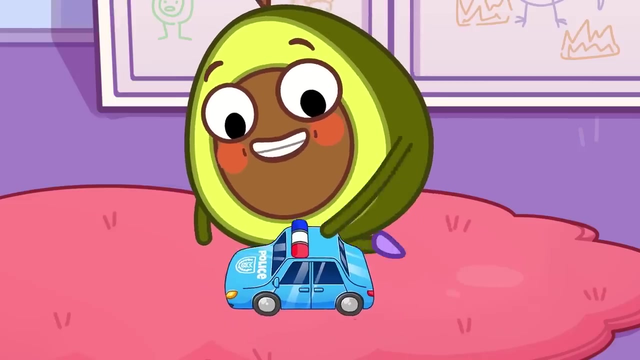 when the light turns green, you can Go, Stop, Go. Remember the rules, kids. A red light means Stop And a green light means Stop. Come on, Let's go. Thank you, Mr Light Pit is playing with his toy police car. 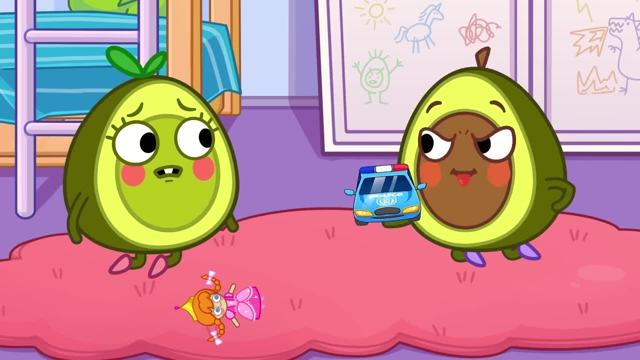 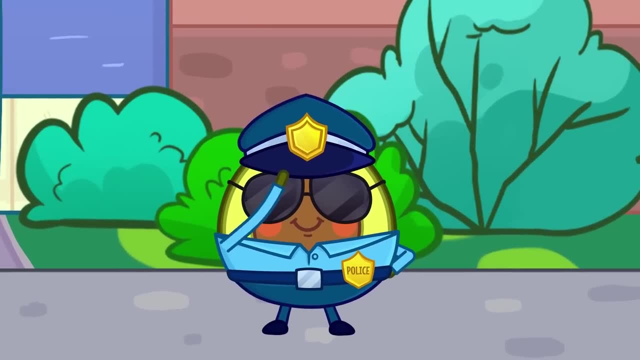 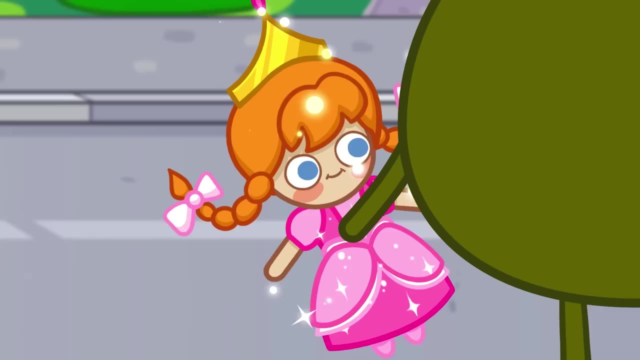 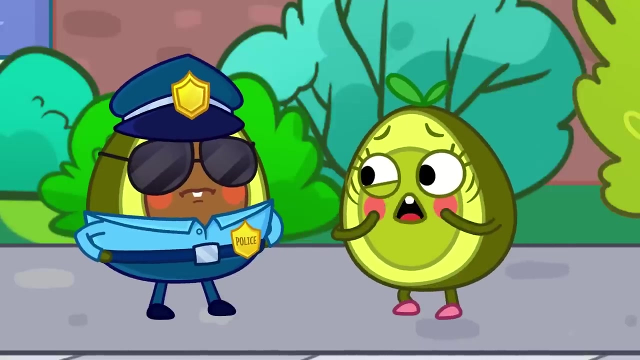 Penny wants to play too. Oh Pit, How should a police officer behave? Hello Officer, Who's that in the bushes? Oh no, Mr Lemon has taken Penny's doll. Ballisman, My doll was stolen, Huh. 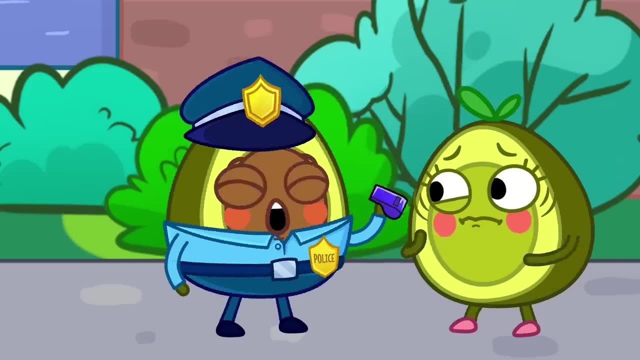 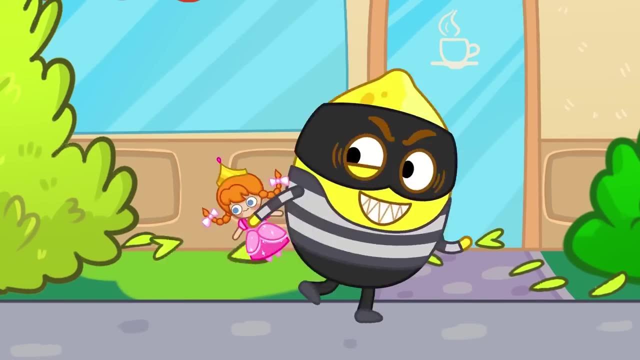 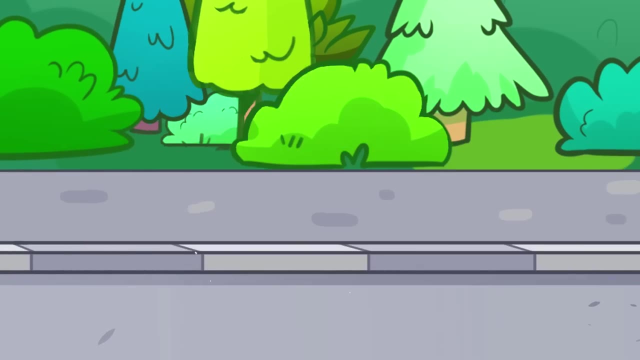 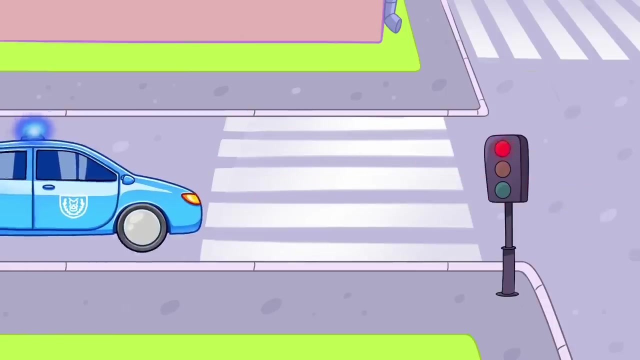 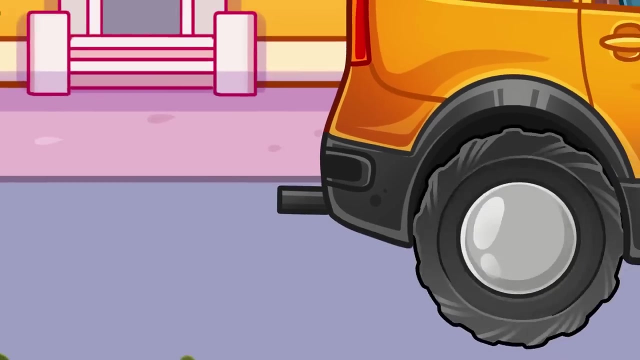 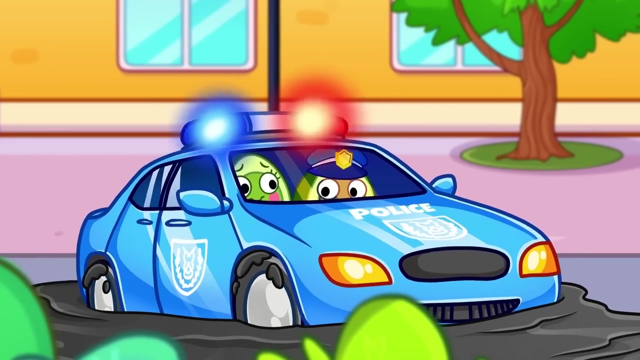 Hmm, Hmm, That's who stole it. Who stole the doll? Do something, Pit. Mr Lemon is getting away, But Officer Pit is on the case. Watch out for the oil. Pit and Penny are stuck, But not for long. 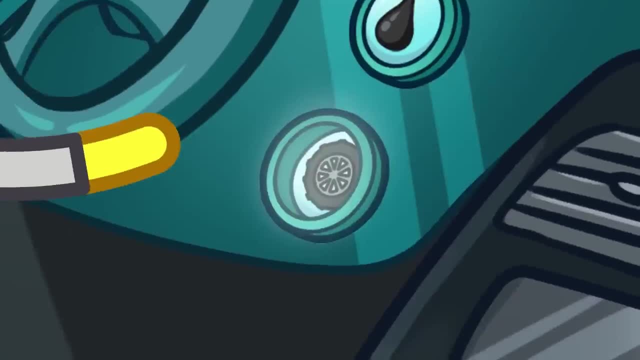 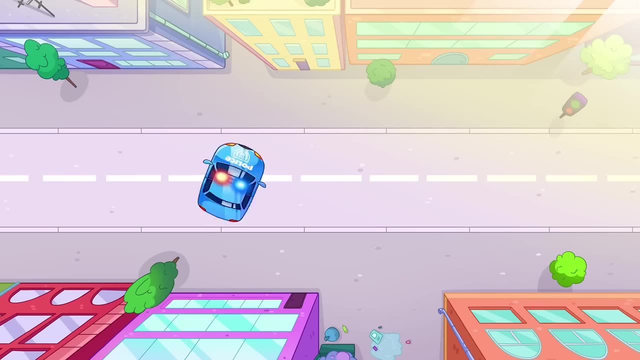 The police are now going outside. Let's head back. Mr Lemon, I think you should watch where you're driving. Nothing for you, Mr Lemon. I'm sorry, Don't let your father die. Mr Lemon is gone. 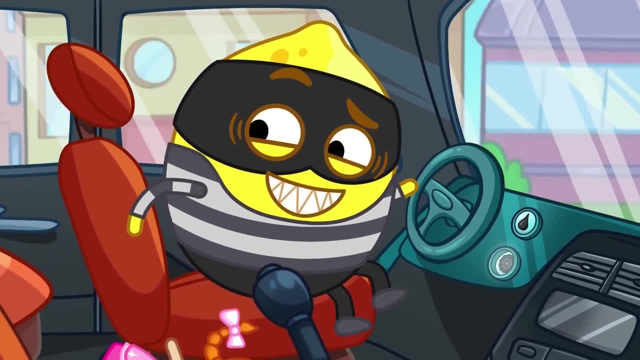 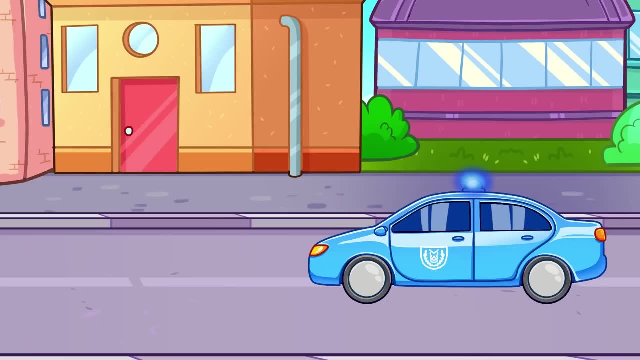 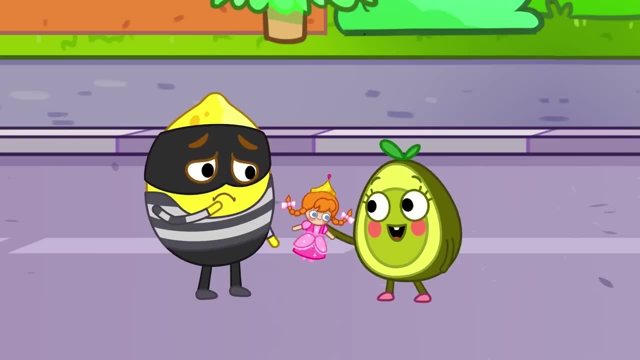 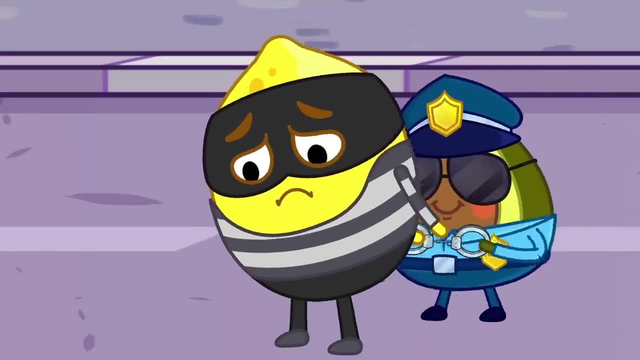 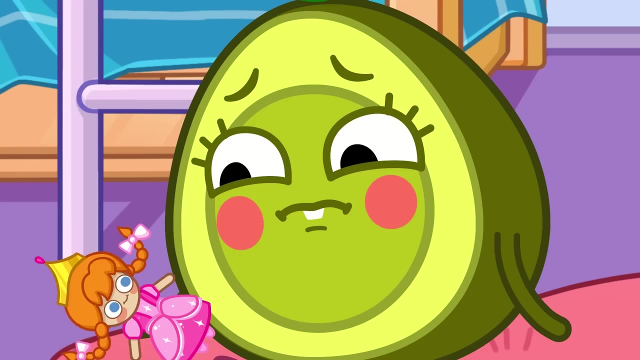 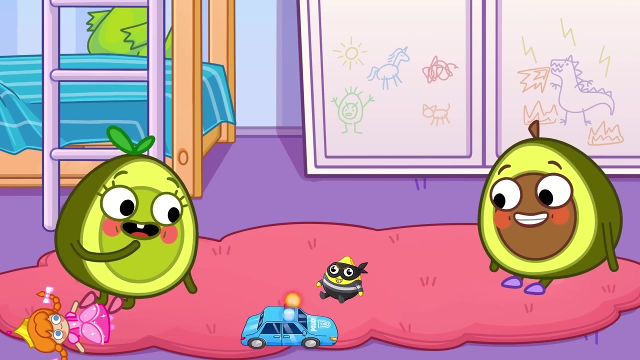 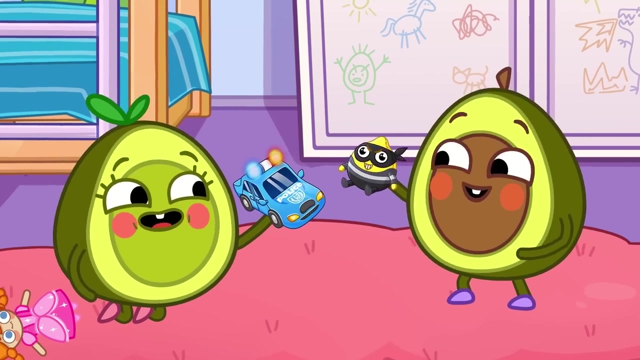 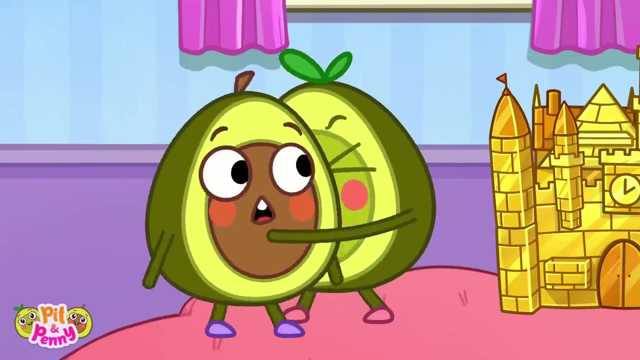 Up ahead, Up ahead, Up ahead. Thank you, Ballisman, for saving my favorite doll. Well done, Officer Pit. Maybe playing with pennies wouldn't be so bad. Have fun. Wow, What a lovely gold castle. Pit wants to play too, but Penny doesn't want to share. 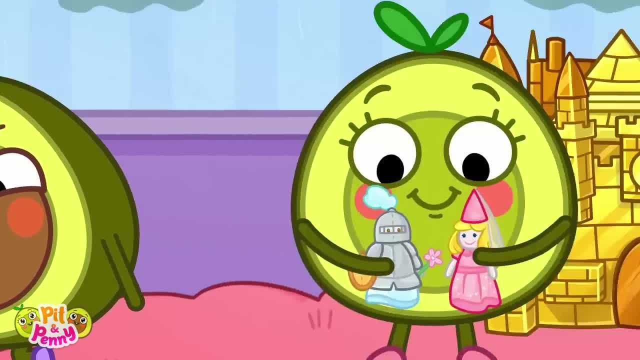 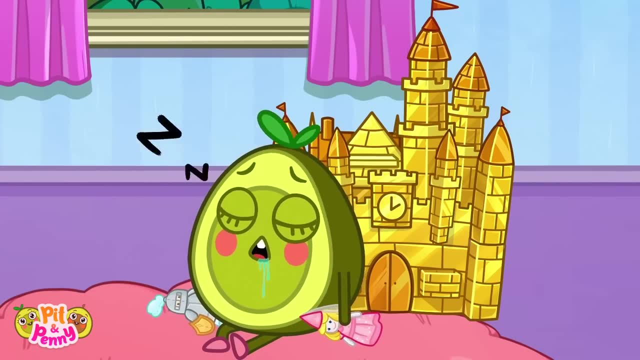 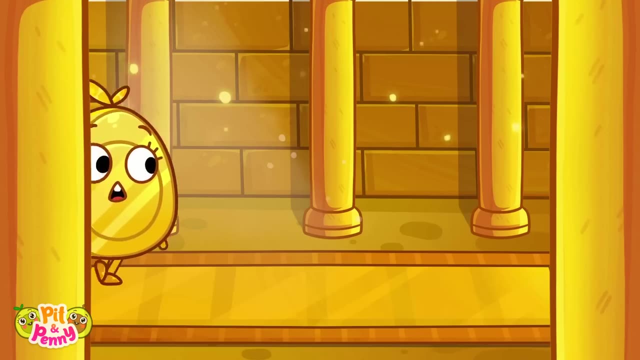 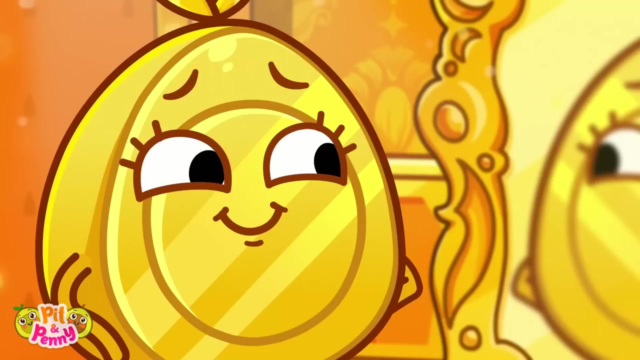 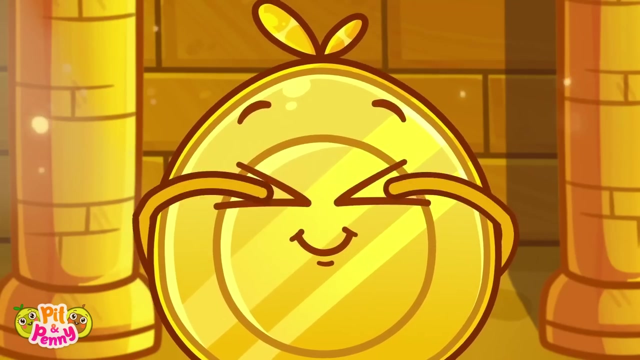 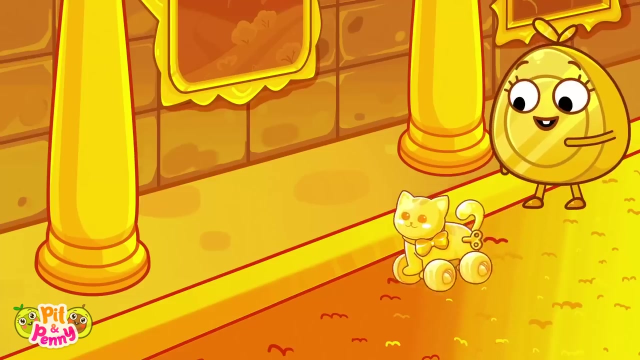 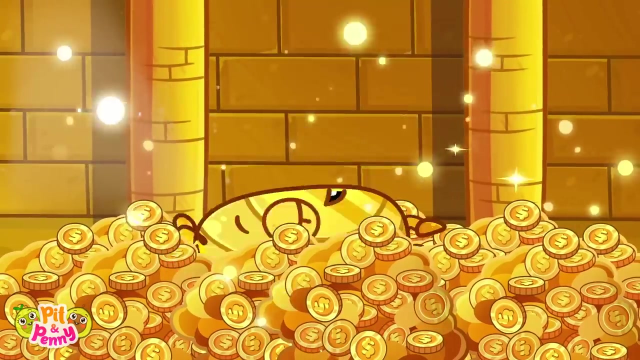 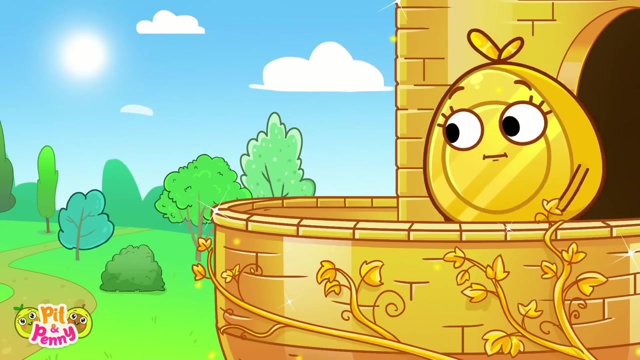 Poor Pit. I wonder what Penny is dreaming about. Look, Penny, everything is gold, Even you. Wind-up Kitty is here. Let's wind her up. Oh, Oh, Oh. Who could that be? You should use a telescope, Penny. 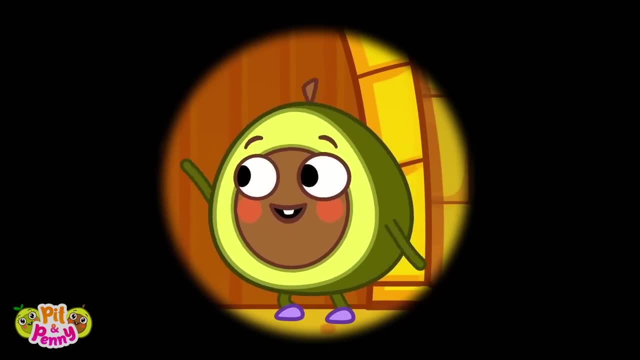 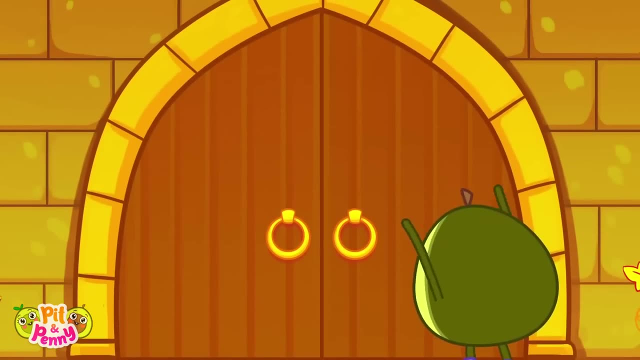 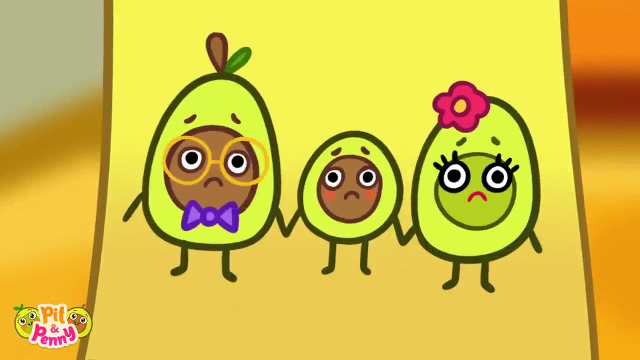 Mommy, Daddy and Pit have come to visit Penny. Your family came to visit you. Will, Penny, let them in? No, Why not, Penny? I can't let you in because you are not golden like me, Penny, You're not golden like me. 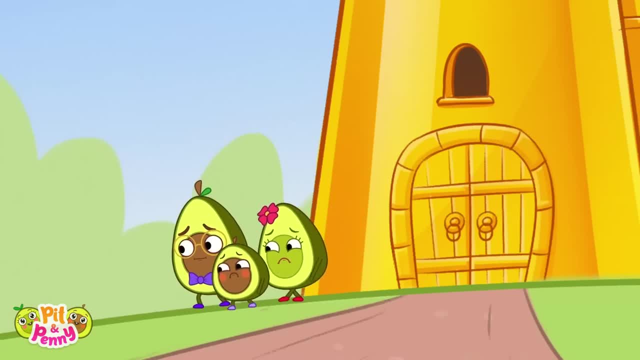 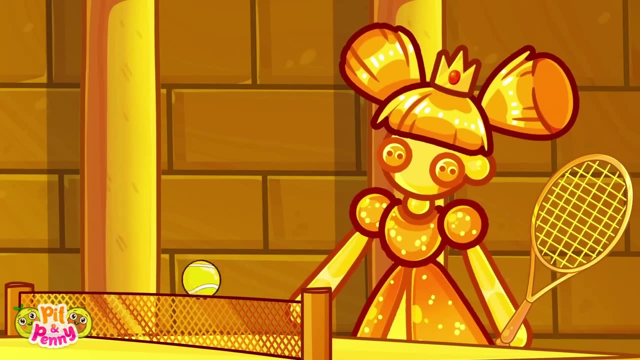 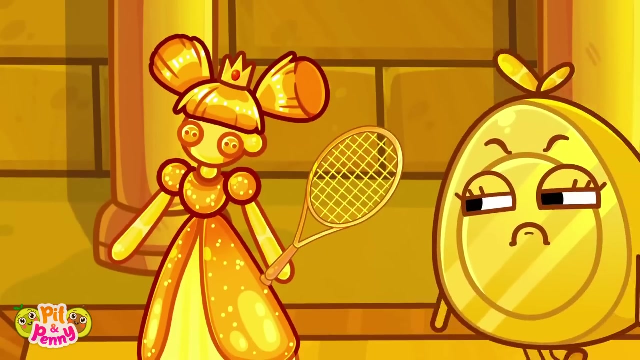 Penny. Sorry, Mommy, Daddy and Pit, Penny Dolls can't play tennis. Penny Dolls can't play tennis. Penny Dolls can't play tennis, Penny. What are you doing there? You're making me mad. 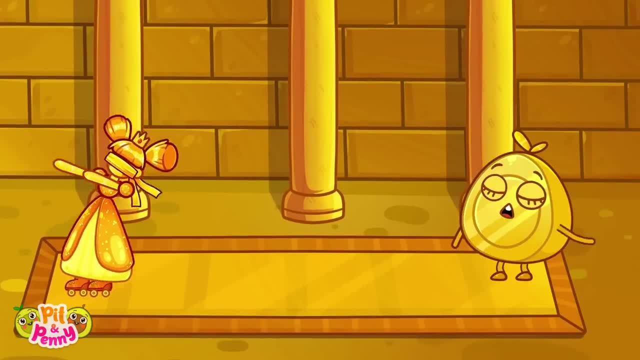 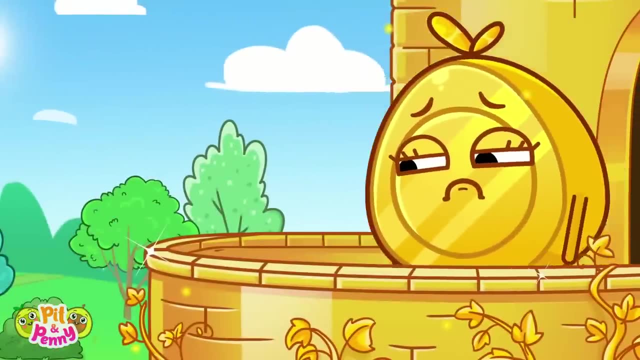 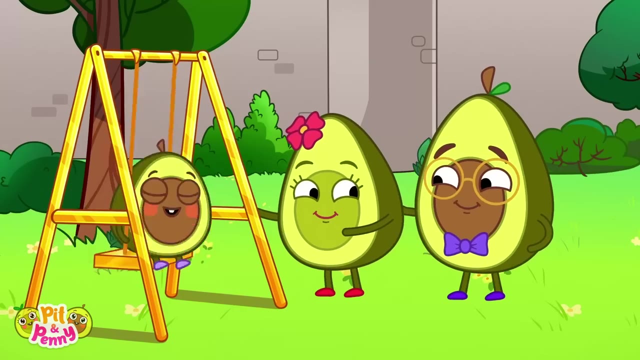 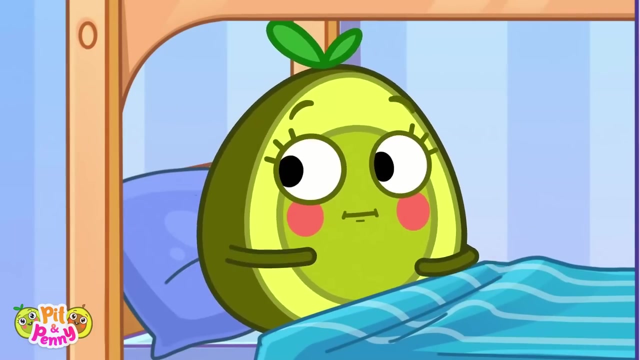 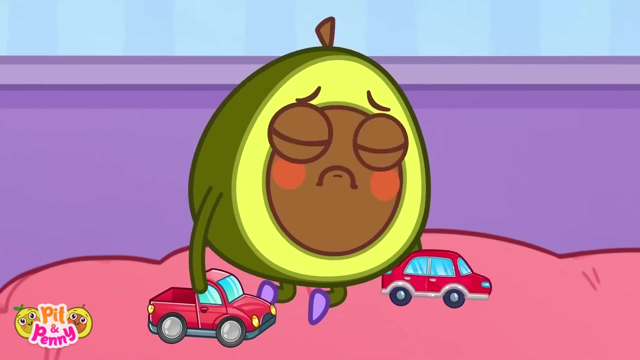 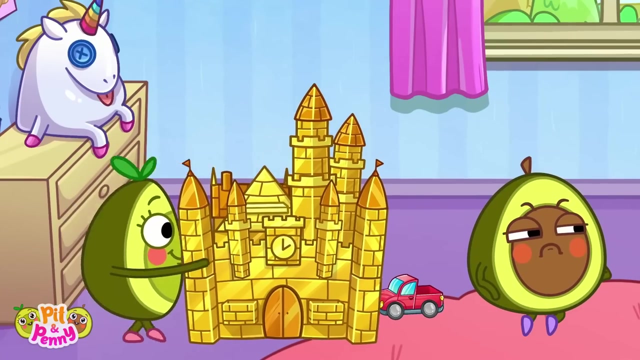 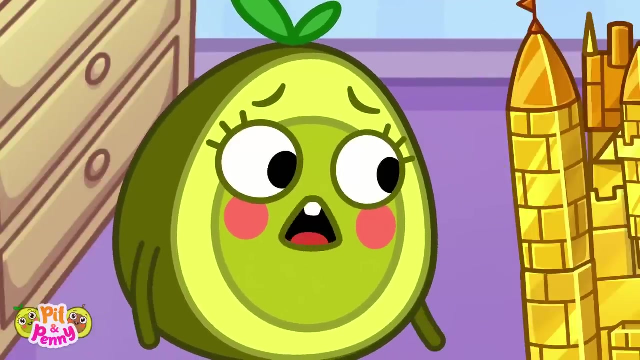 Penny, Penny, You're making me mad. Penny And dolls can't play hide-and-seek. I bet they're having fun. Wake up, Penny. Penny has an idea. Do you have something to say, Penny? I'm sorry, Pit. I realize that it is necessary to share toys. 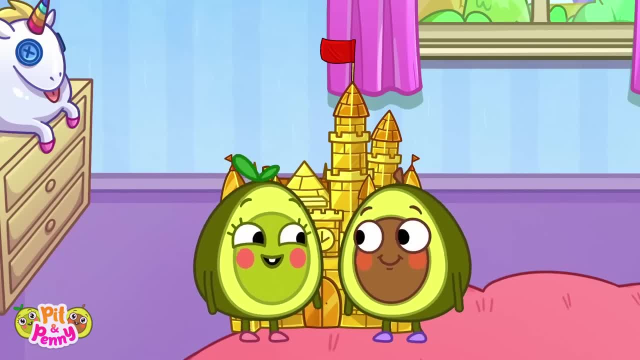 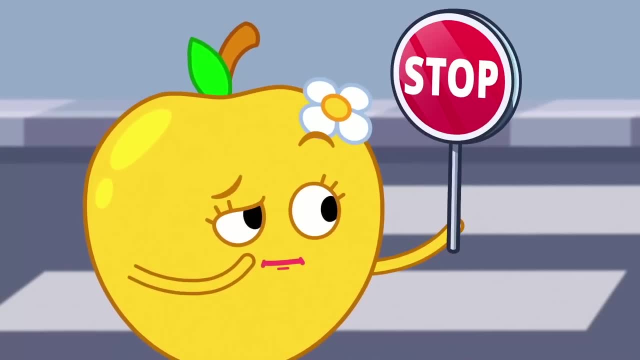 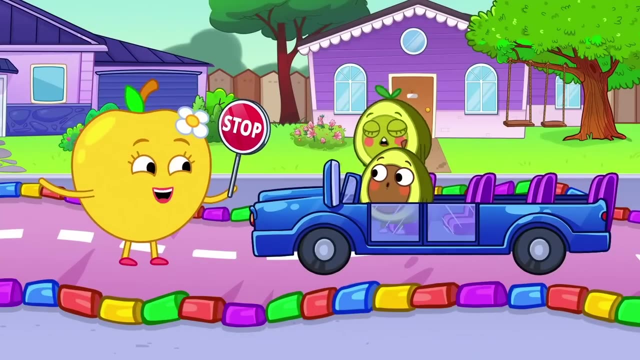 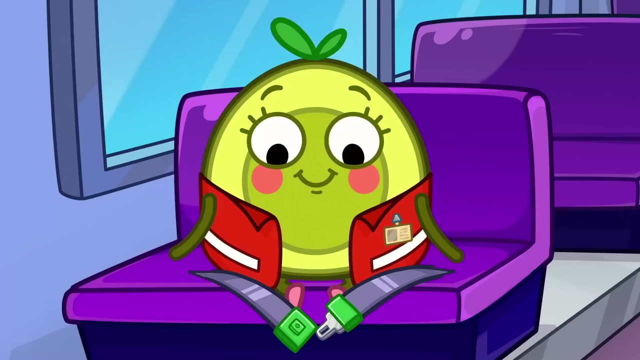 It's always more fun when you share. Here comes the bus. Oh no, Penny, Remember, always fasten your seatbelts. Why are seatbelts important? They keep you safe in an accident. Here comes the bus, Here comes Cherry. 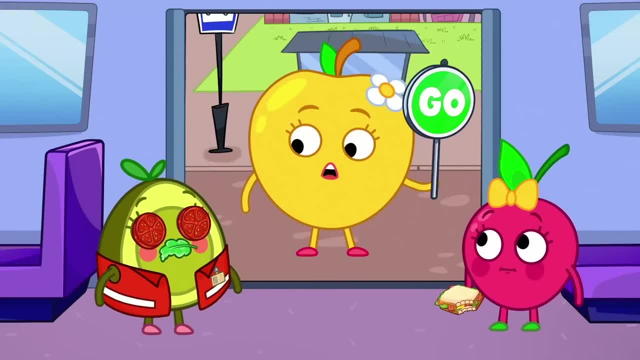 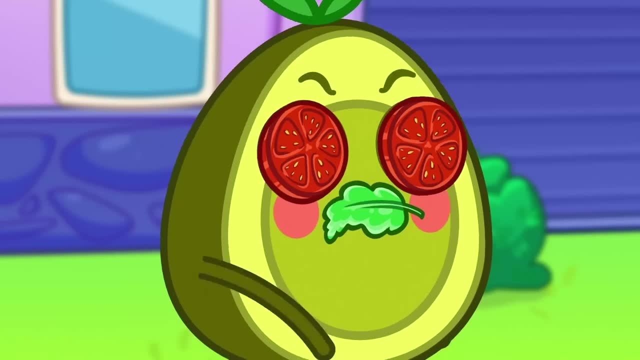 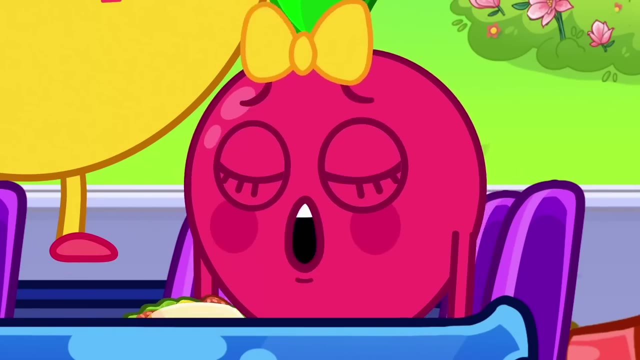 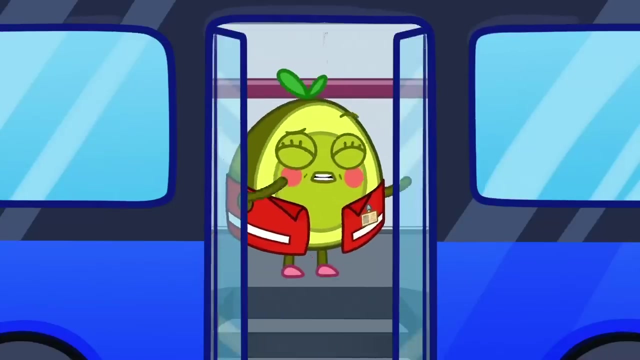 Oh no, Look at Penny Kids. what rules do we have? Do you know? Penny, Don't take food on the bus. It's messy. Sorry, It's blueberry. Take your seat, She can sit with her friends. 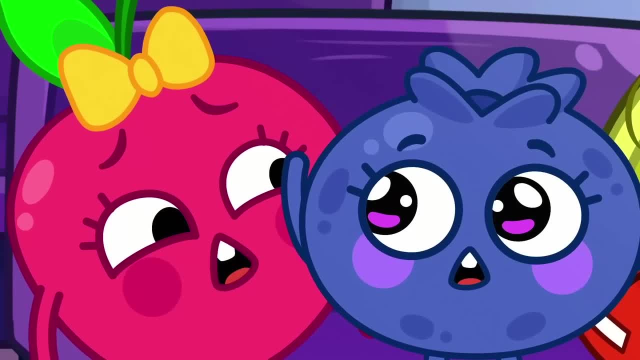 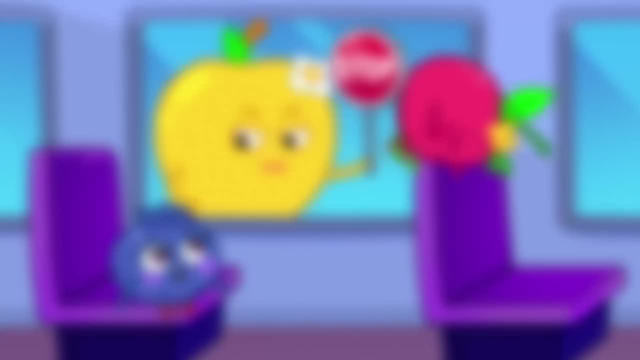 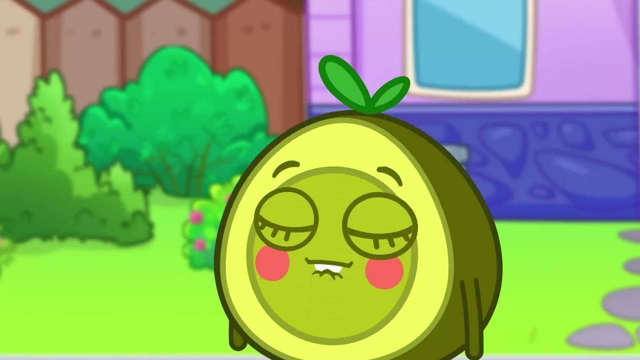 No, that seat is full. You're gonna crush us. I'm almost there. Maybe Miss Apple can help Penny. what do the bus rules tell us? No more than two people. No more than two people. Let's take over. 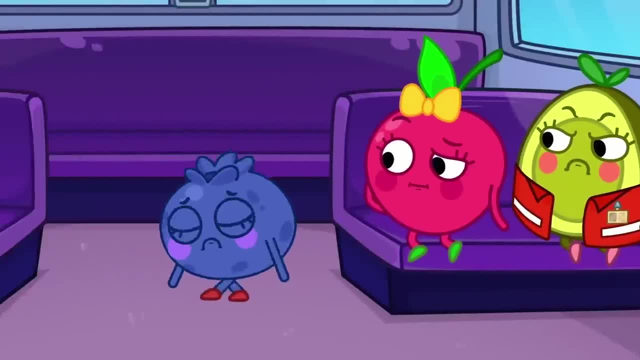 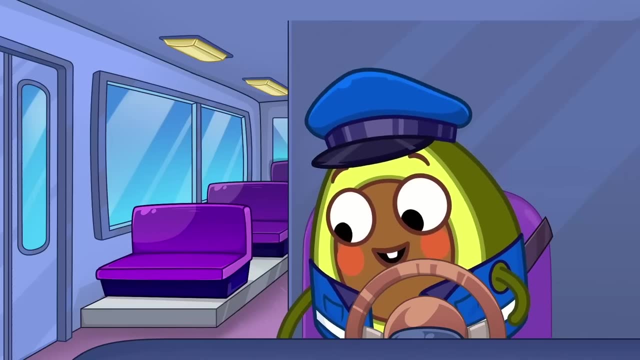 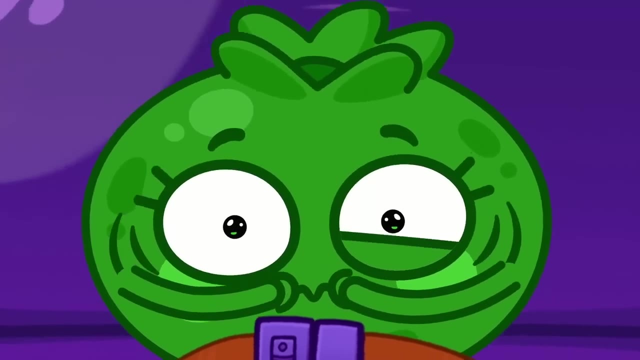 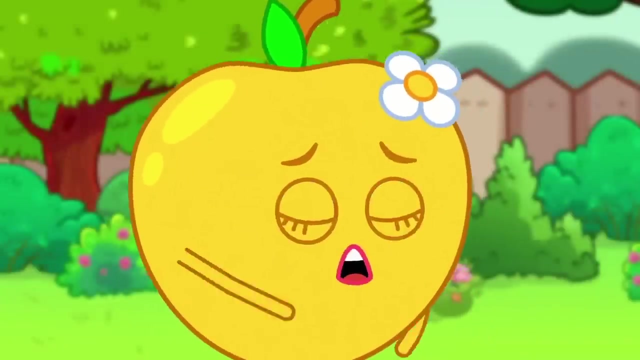 No, don't get involved with서eat. Then where can Blueberry sit? Herewhere she has a seatbelt. cathedral Pete, we have to stop. Blueberry doesn't feel well If the driver doesn't stop. push the stop button. 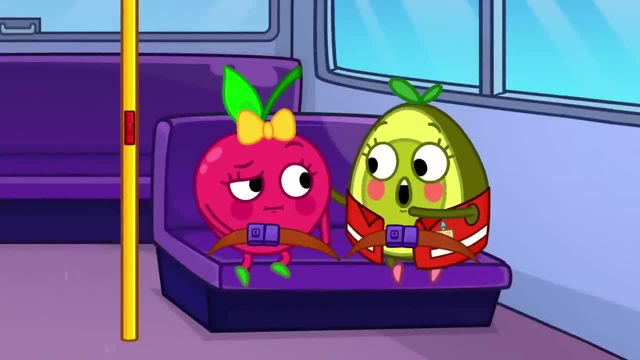 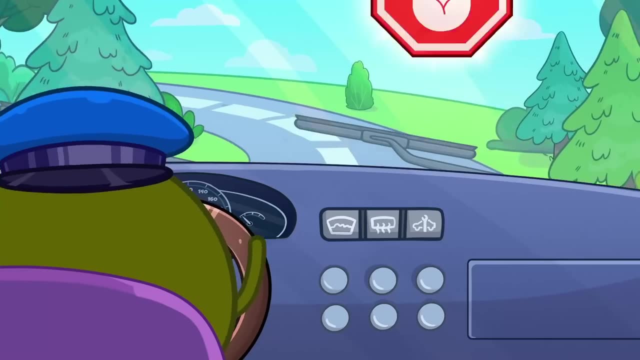 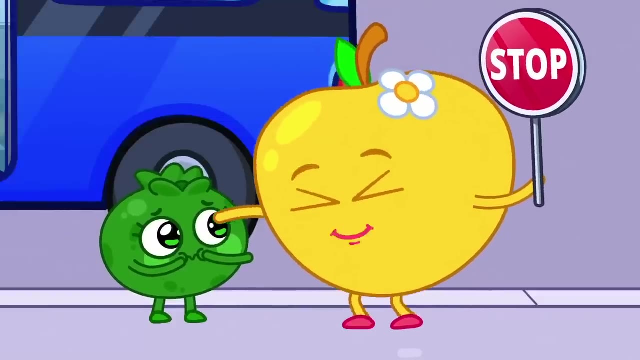 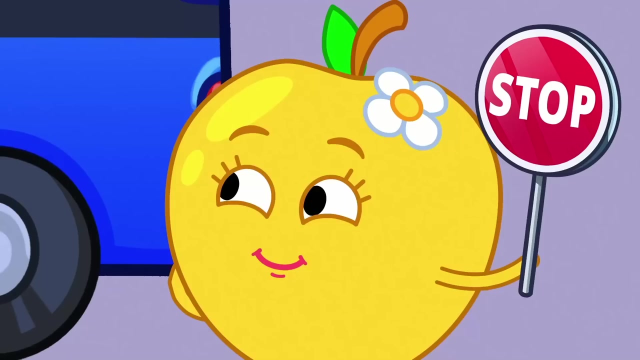 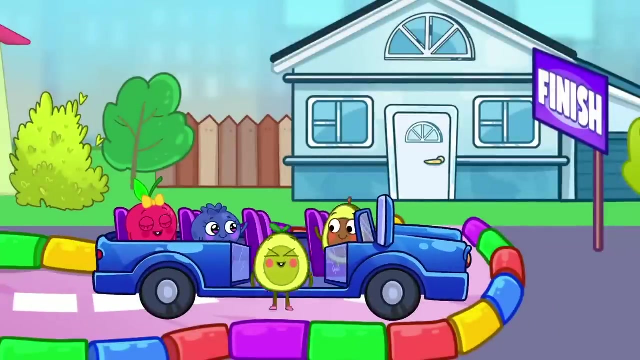 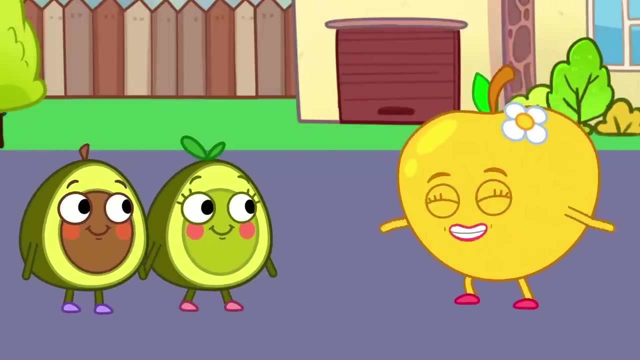 Stop buttons are on the handrails. It lets the bus driver know to stop. Phew Blueberry feels better. Following rules keeps us safe. So have you learned the bus rules? The kids know what to do now. Oh, What do you want to learn next time? 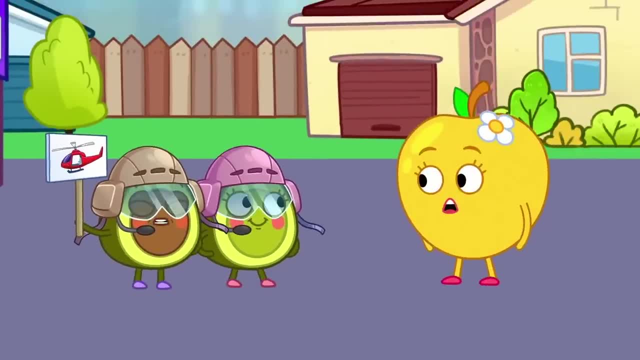 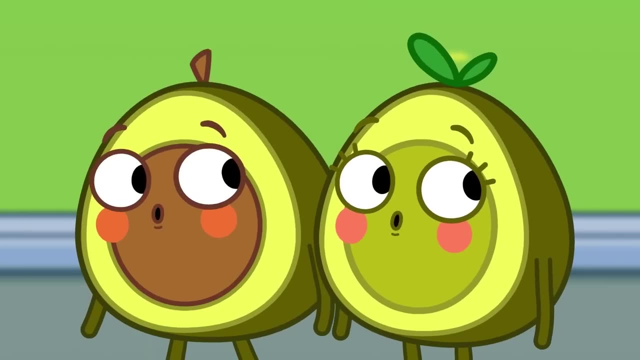 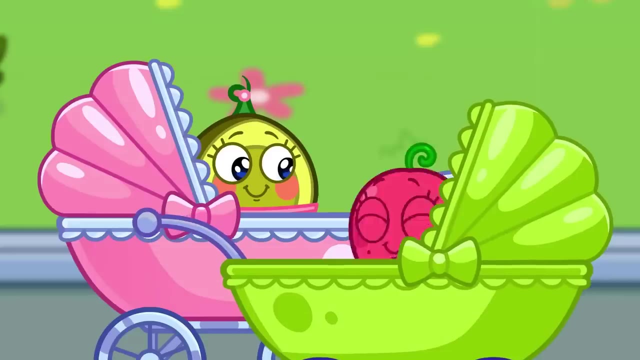 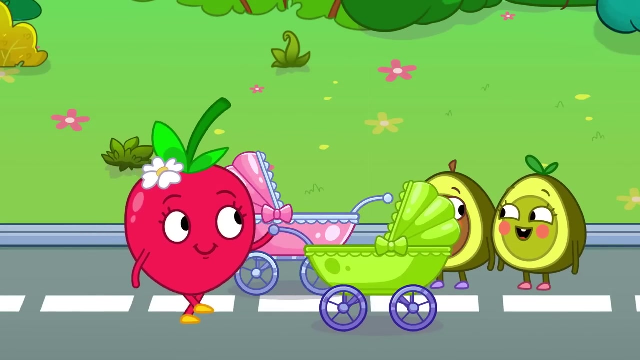 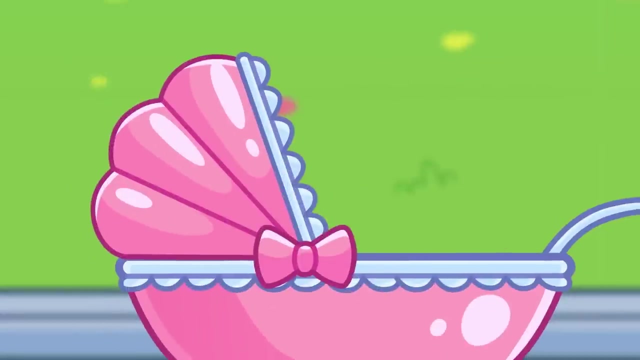 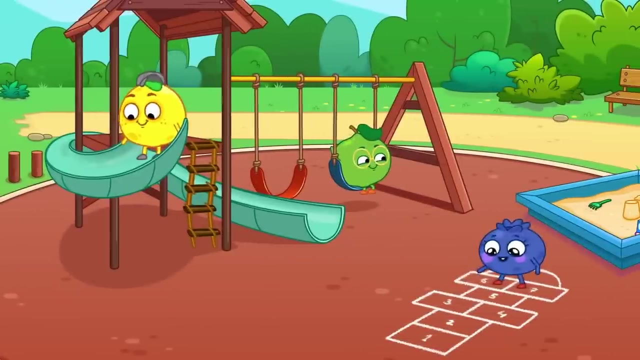 Pit How to fly a helicopter. Oh, Pit, Pit and Penny are taking care of babies. Ooh, Ice cream, Yum. Better check on Baby. Oh, no, Baby got lost. Pitcher, Should she be in the playground? 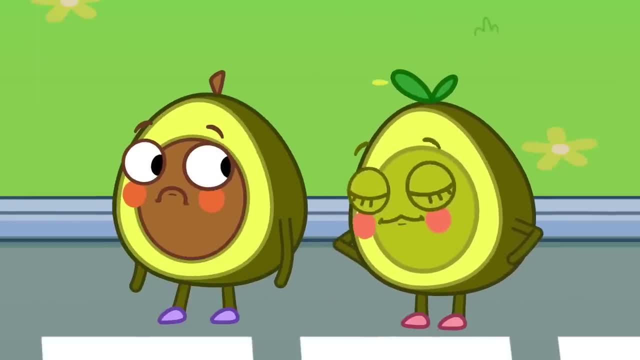 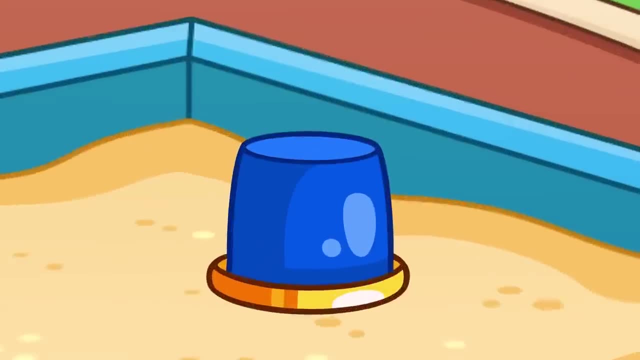 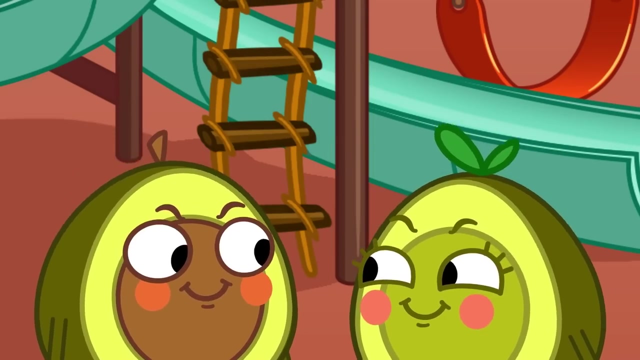 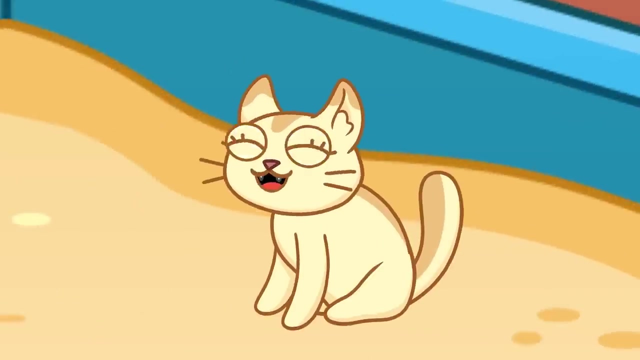 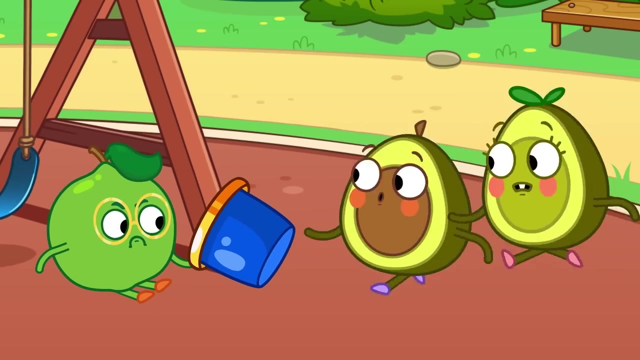 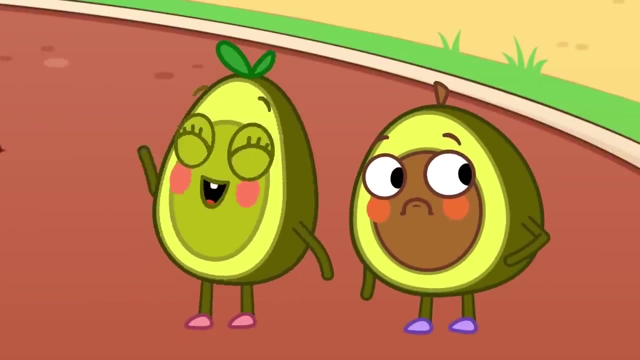 To find a baby, we need to think like a baby. Maybe she's under the bucket. It's just a cat. It's just a cat. It's just a cat. Oops, You hit Lime with that bucket. Maybe Baby is on the slide. 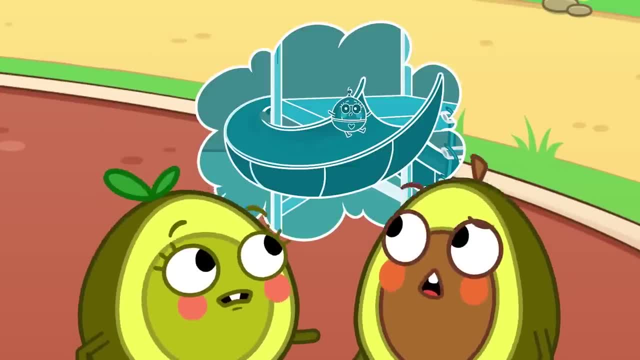 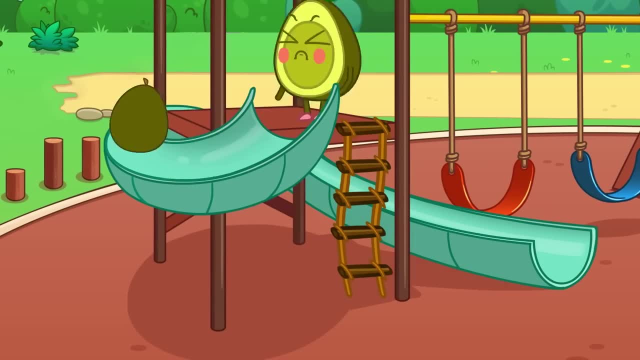 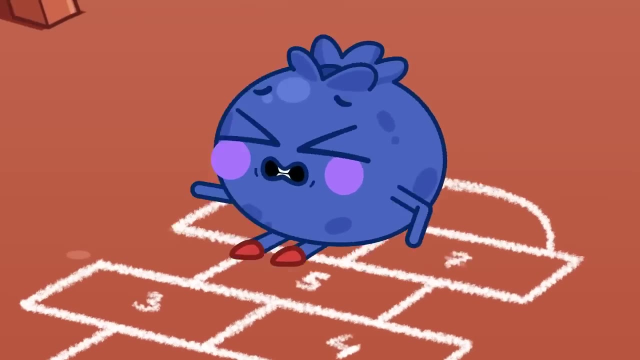 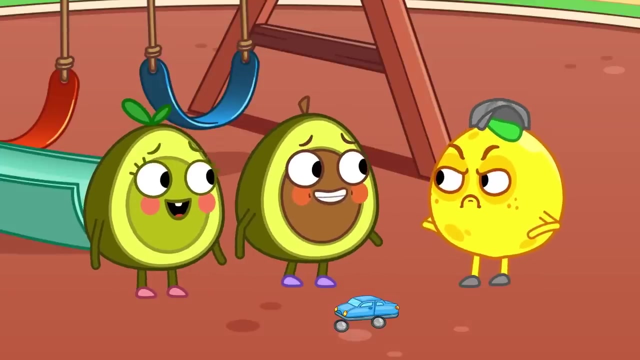 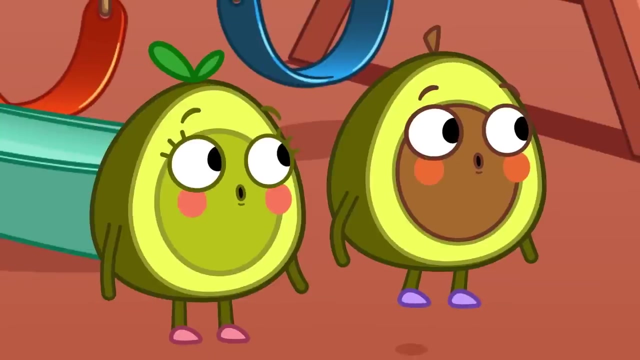 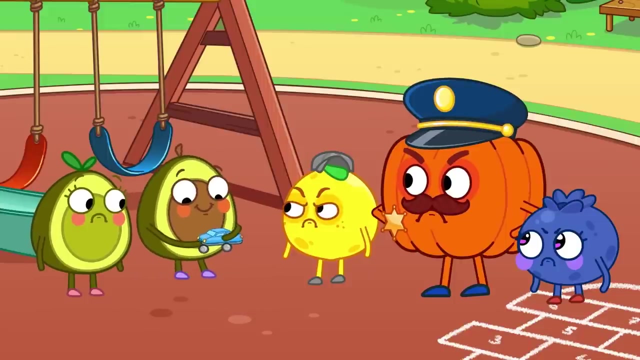 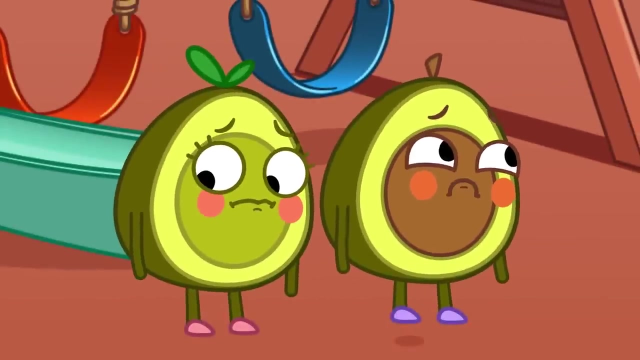 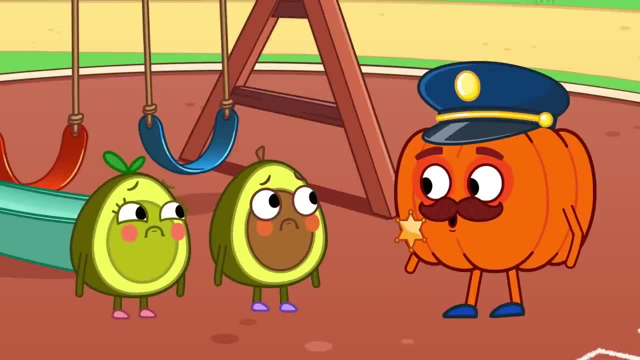 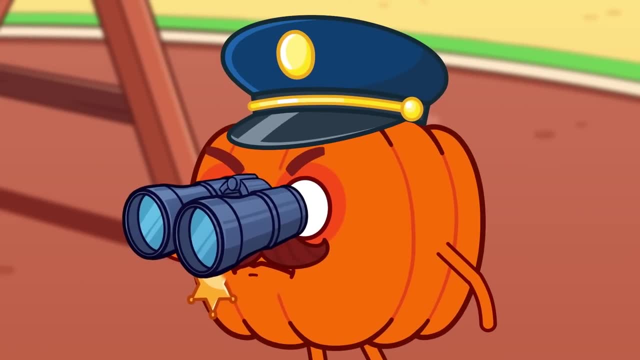 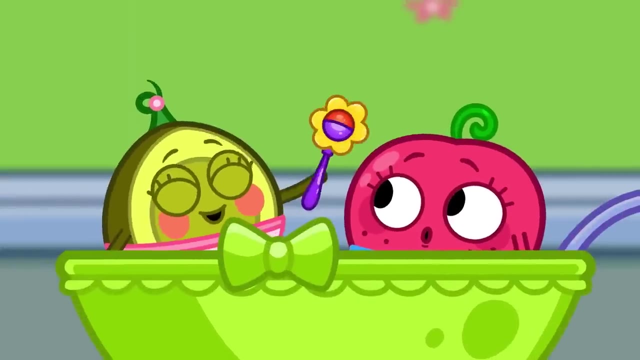 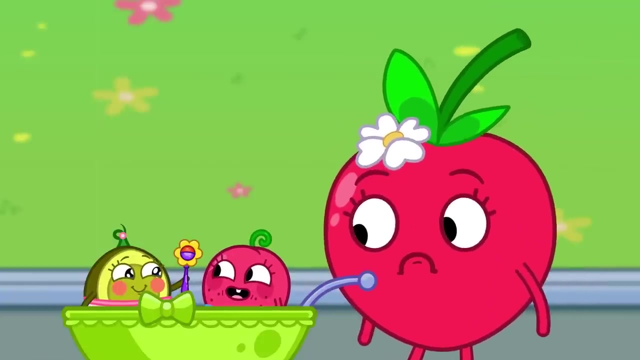 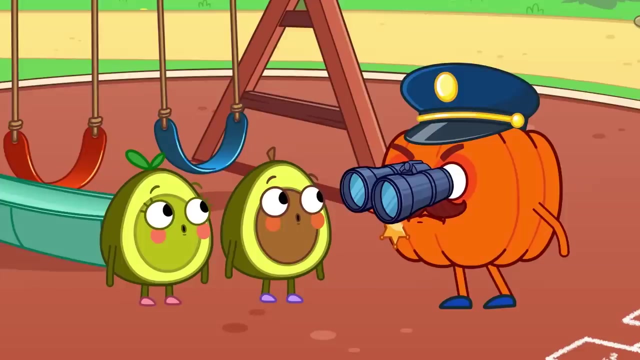 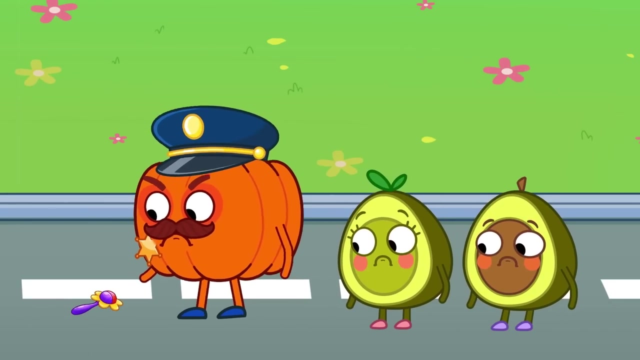 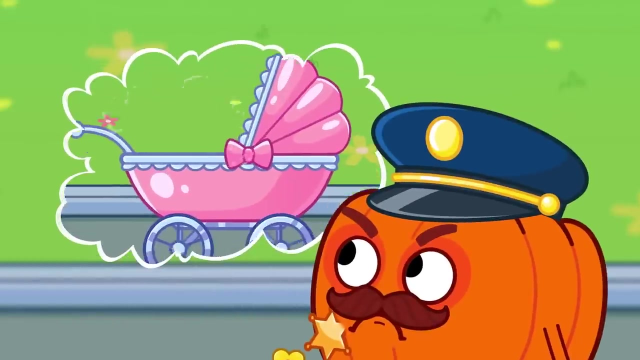 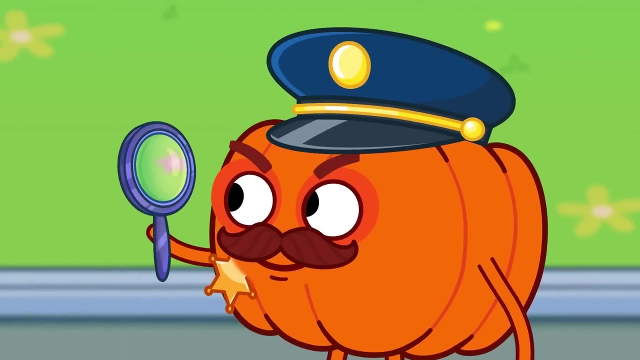 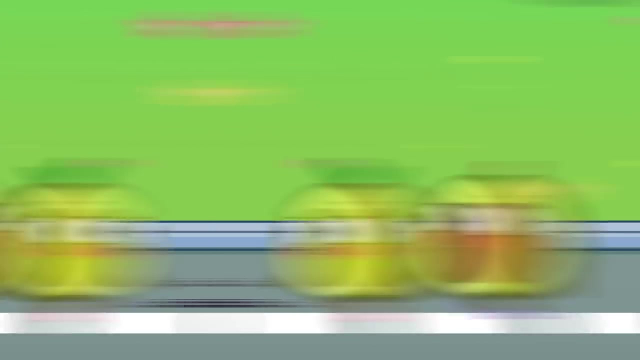 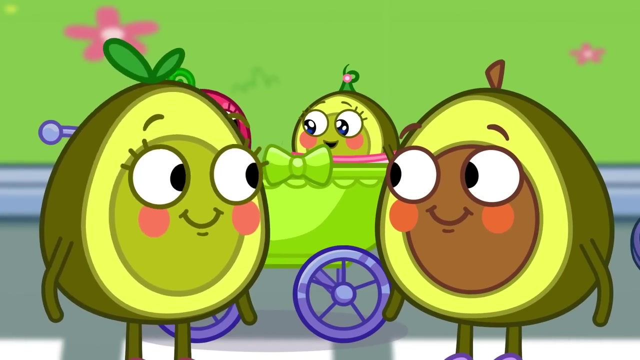 I will help you. Let's look for a clue. Oh, We're a bit in pain. There's Baby's rattle. Did someone take Baby Tire tracks? Let's follow them. We're found. Baby Pit has something to say. 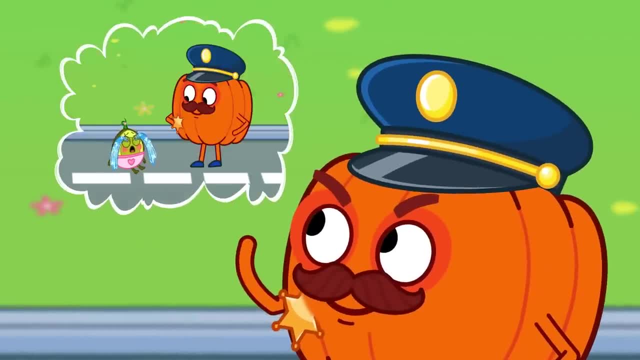 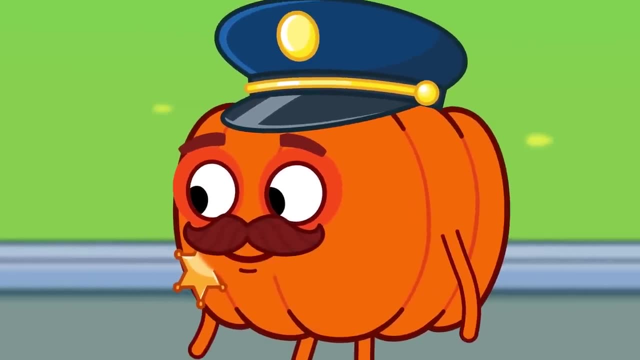 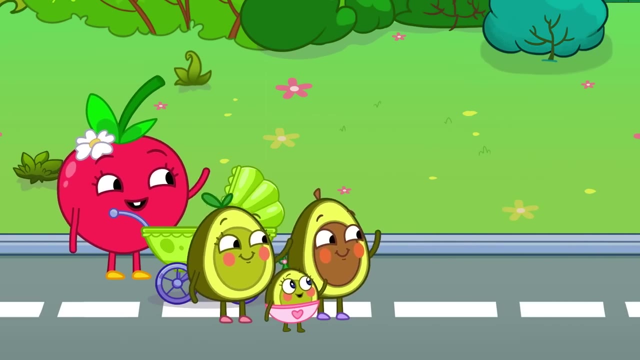 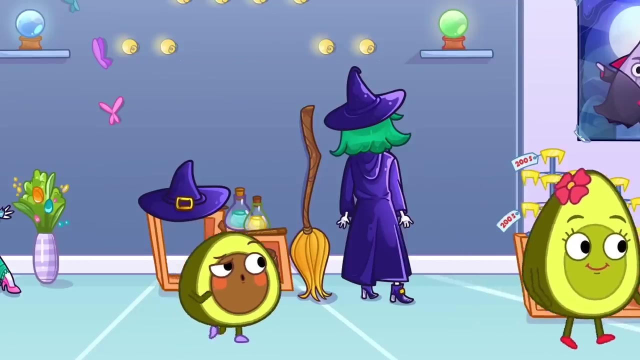 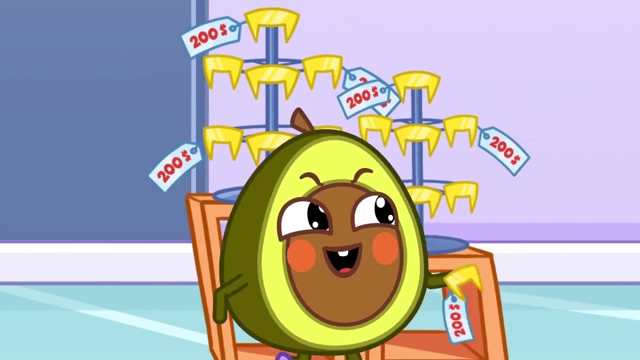 Thank you. If you get lost, always contact the police. They will get you home safely. Bye-bye, Officer Pumpkin. It's time to buy the costume for Halloween. I can be a vampire, And those gold teeth are perfect Oh. 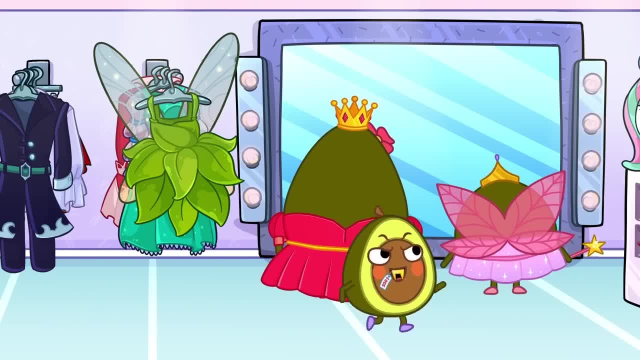 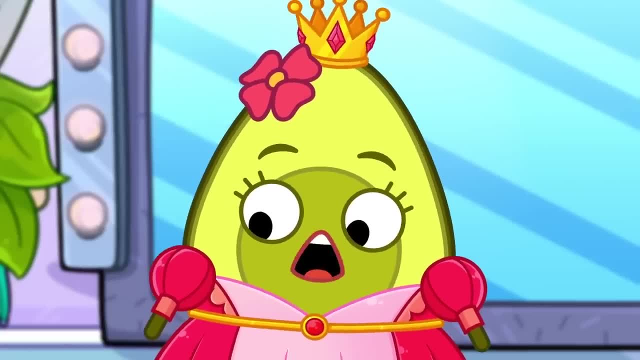 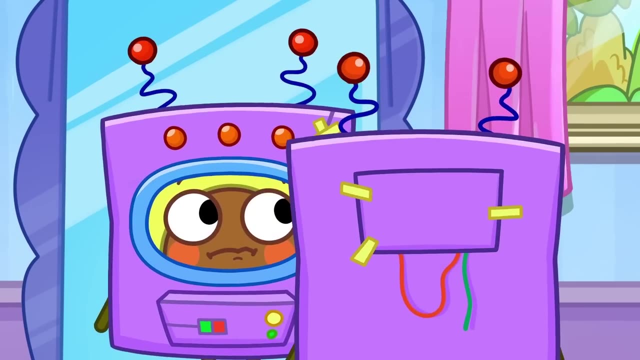 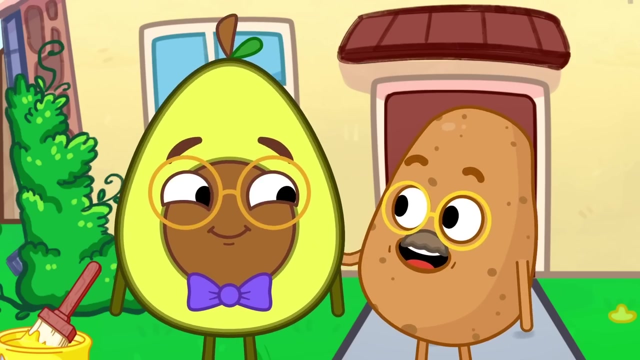 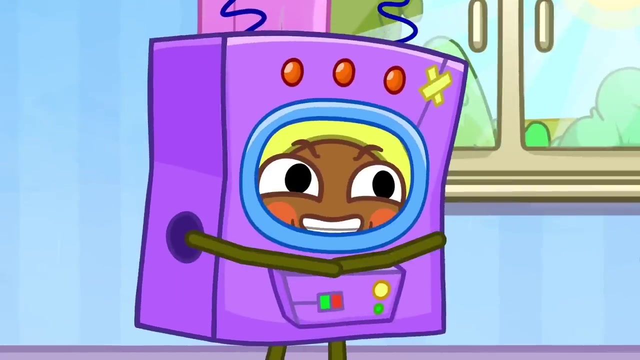 Let's scare Mommy and Benny. Oh Pit, it's too expensive, Aww, but I need gold fangs. Being a robot is boring Gold fangs. I'll paint my teeth gold, Got it? Shhh, Da-da-da-da-da-da. 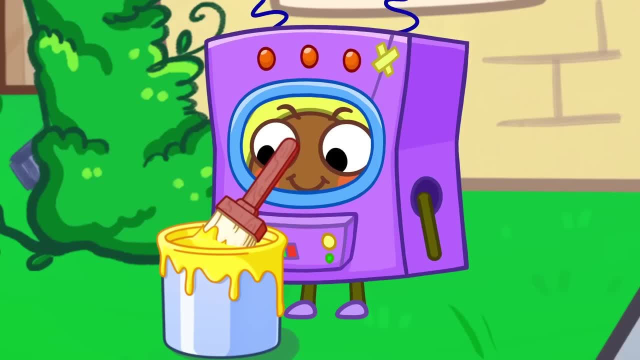 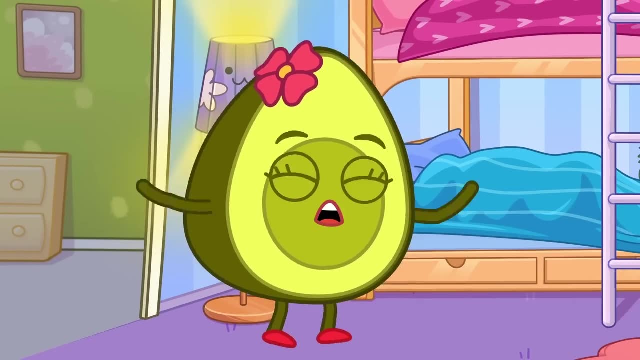 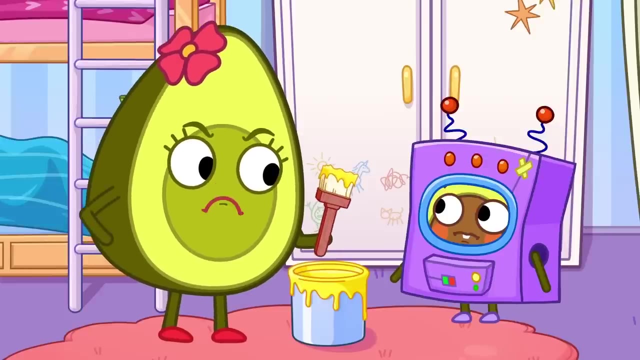 Da-da-da-da-da-da-da, Da-da-da-da-da-da-da-da-da, Da-da-da-da-da-da, Da-da-da-da-da-da-da-da, Aww, Pit, It's. paint is for wood. It's dangerous to put it in your mouth. 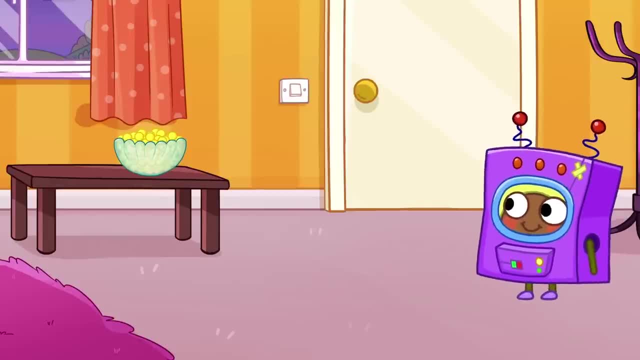 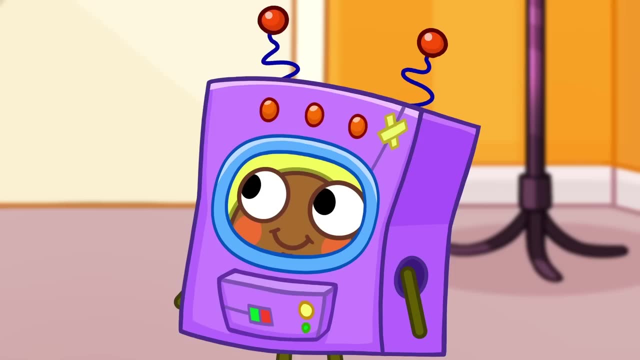 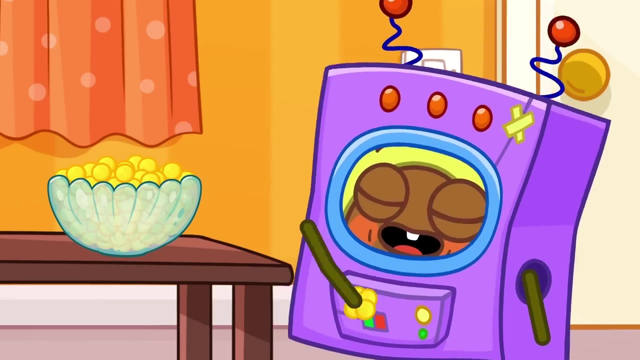 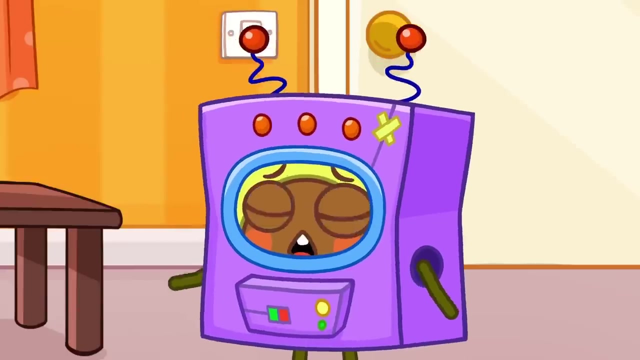 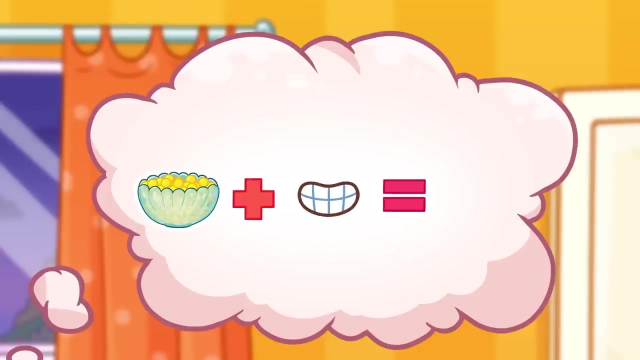 Okay, Gold candy. That candy will turn my teeth gold. Hehe, Pete, don't eat too much candy, Your teeth will be hurt. I just wanted to be a vampire with golden teeth. Oh no, I don't want cavities. 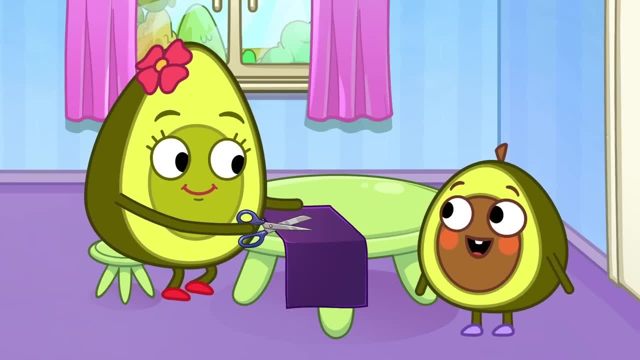 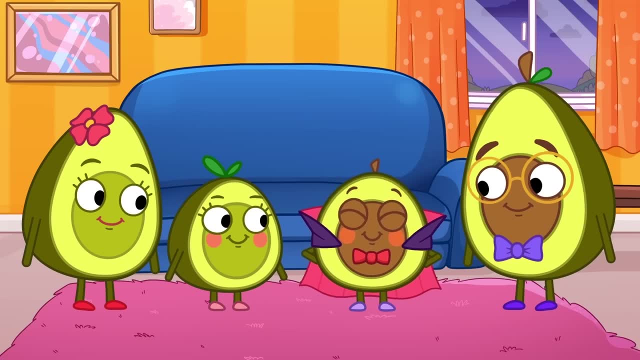 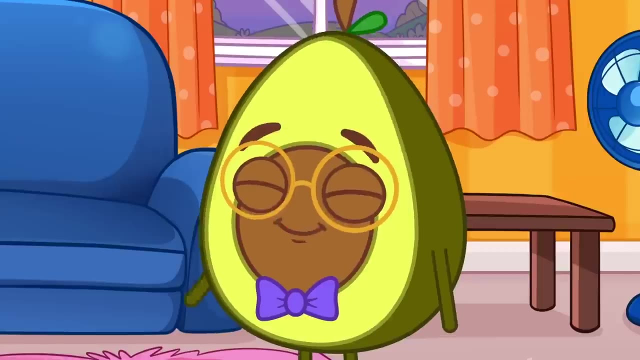 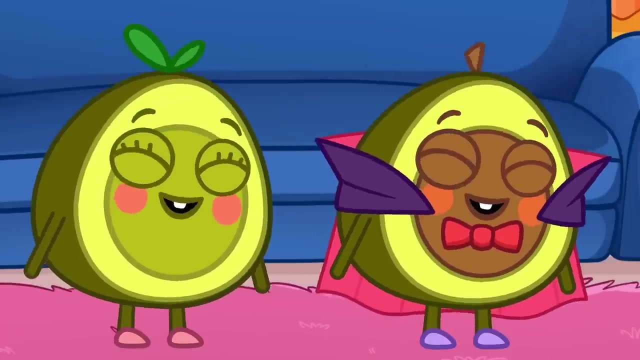 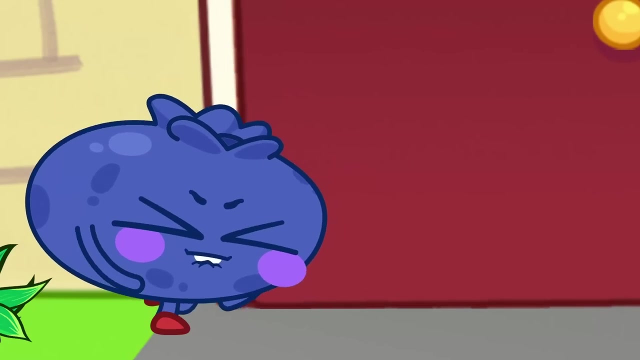 I have an idea. And now for my teeth Ready, Pretty cool. Remember kids. White teeth are always better than yellow ones because they are healthy. Cherry and Blueberry have come for a visit. Don't kick the door. What should you do, Cherry? 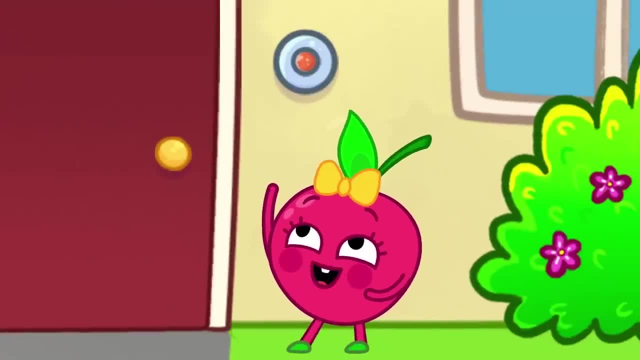 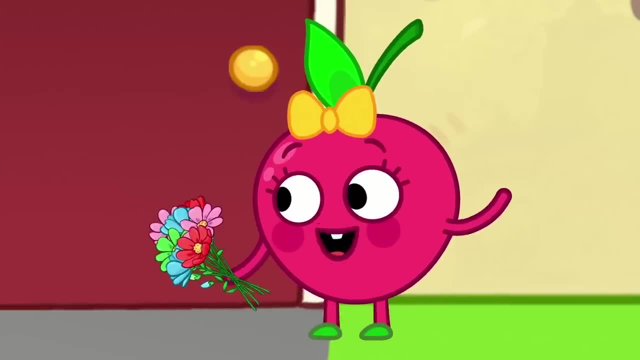 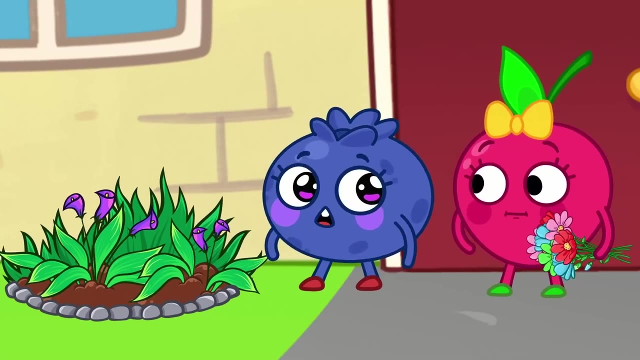 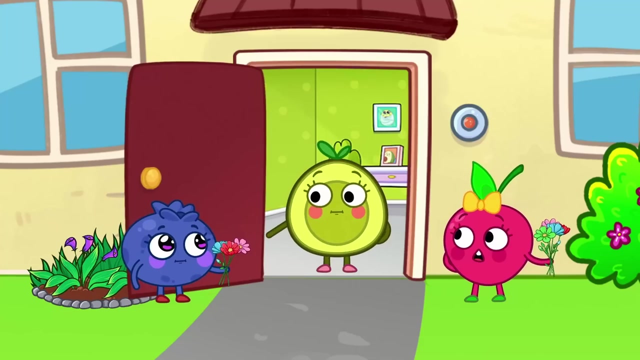 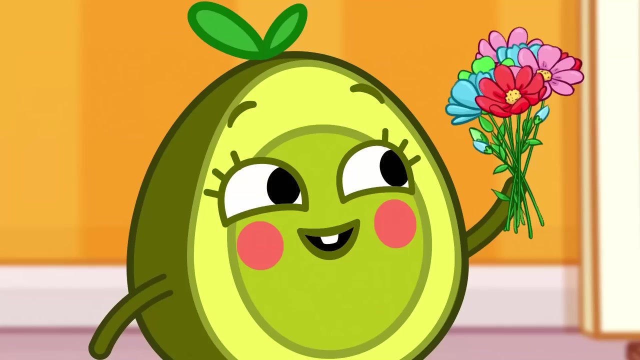 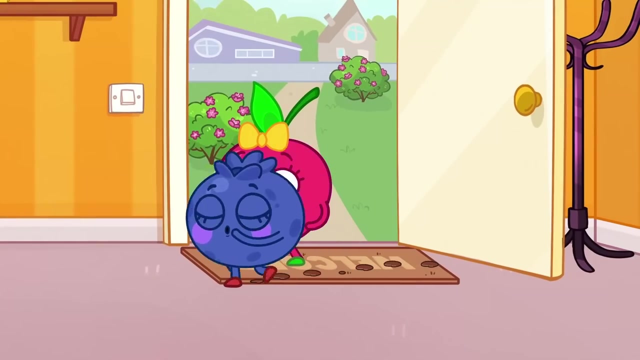 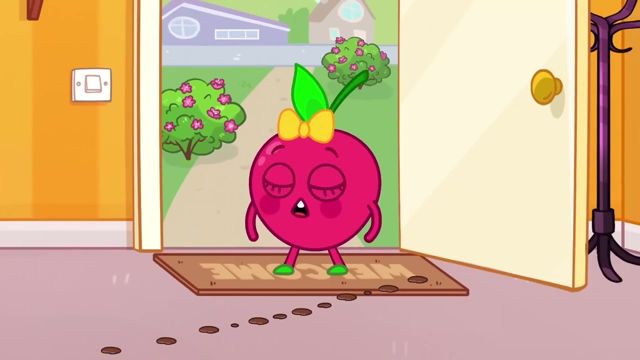 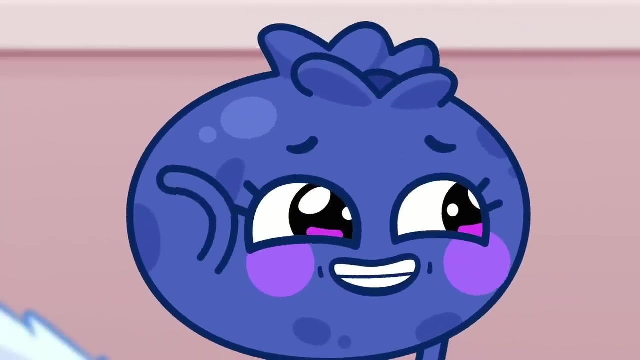 Be quiet, Better use the doorbell. What are the flowers for? Don't forget to bring a gift. Never pick flowers from someone's garden. Hello pennies, Blueberry has muddy feet. What should Blueberry do? Wipe your feet before coming inside. 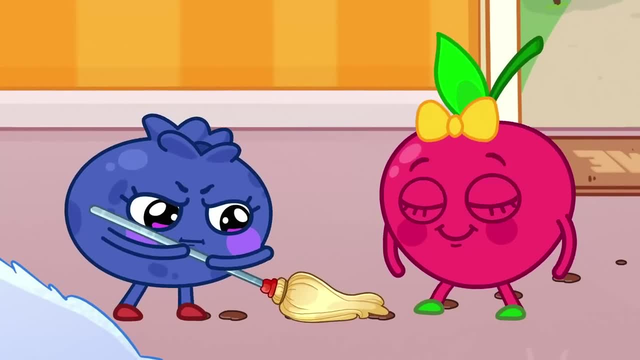 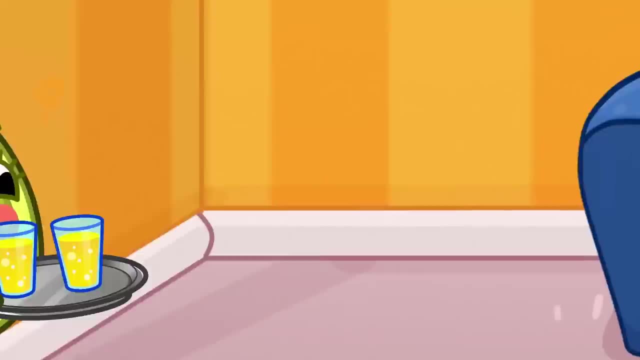 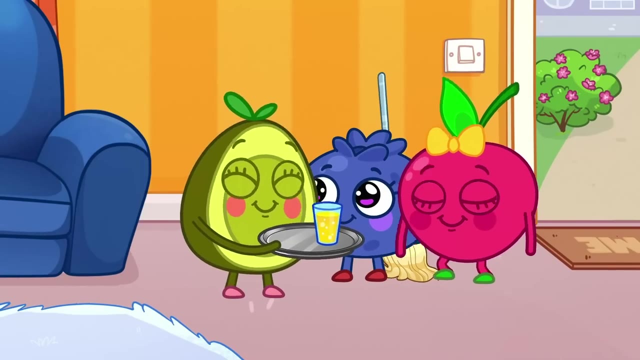 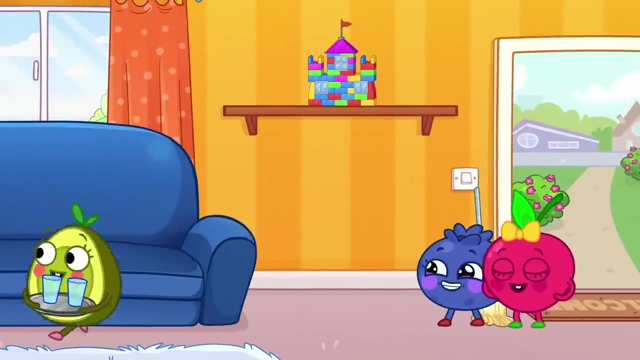 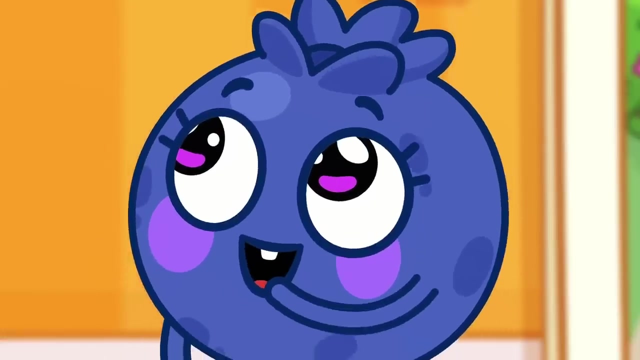 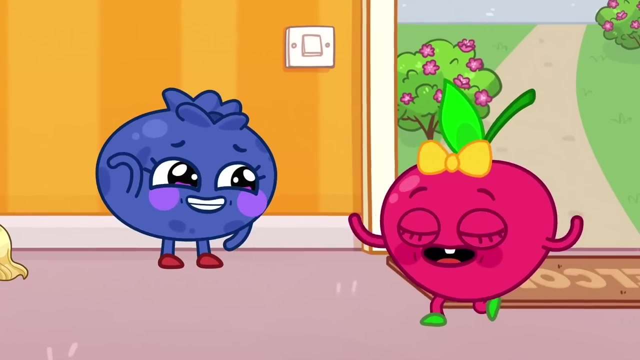 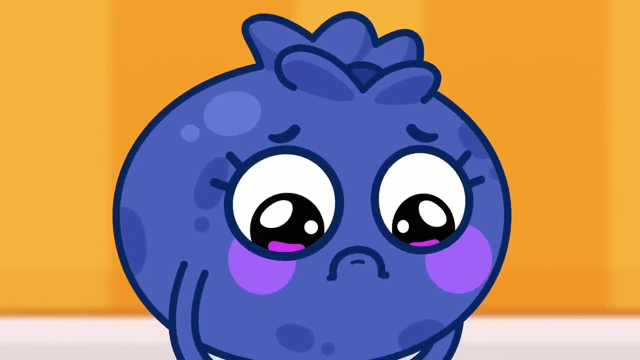 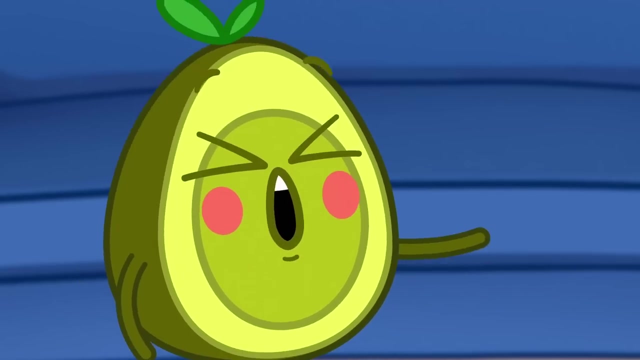 You better clean that up. Well done, Blueberry. Do you want some juice? What a cool toy. Blueberry broke it. Don't touch toys without asking. Oh no, What's wrong? Penny, I forgot to show you my new toy. 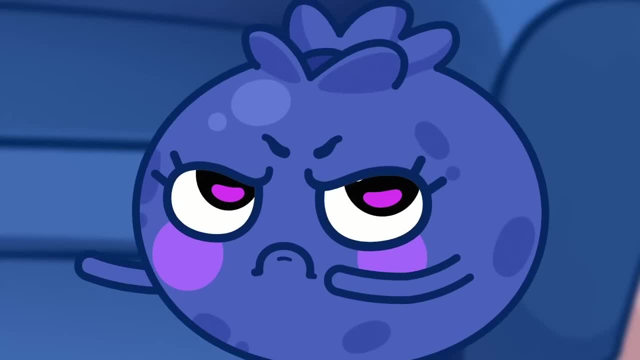 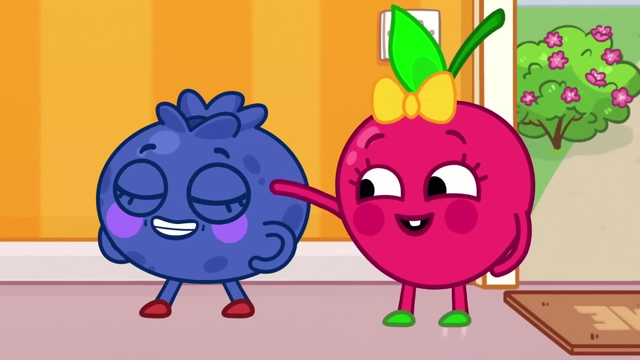 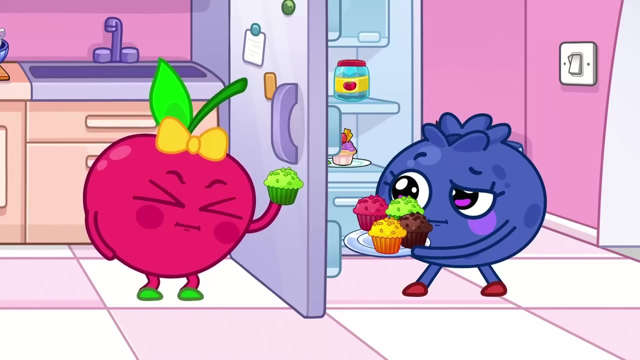 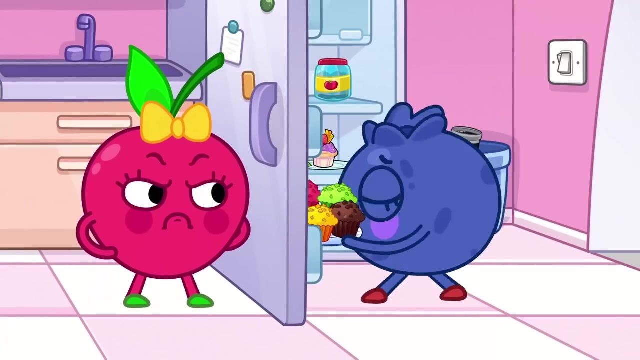 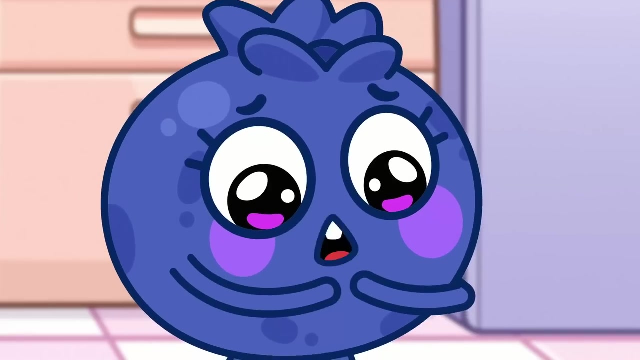 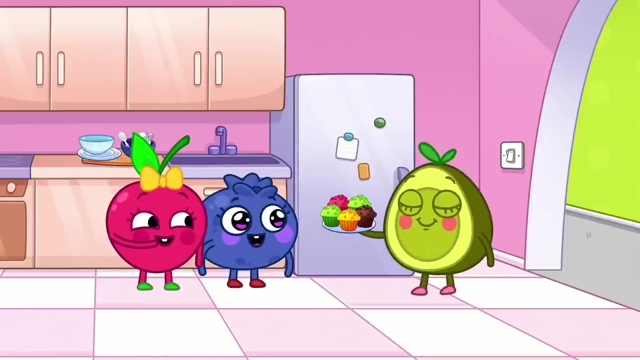 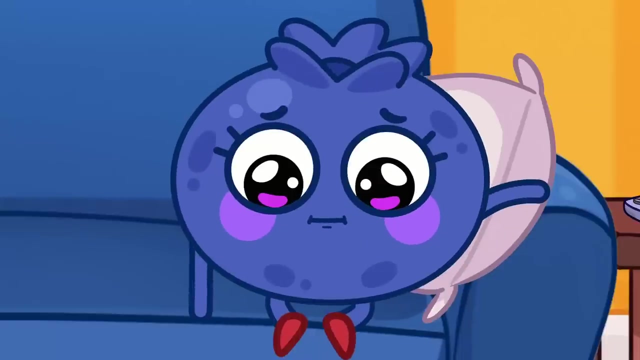 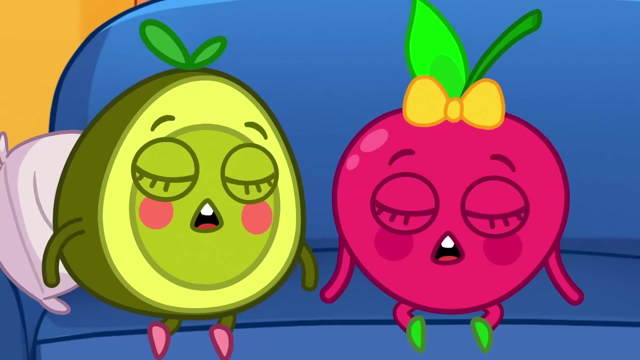 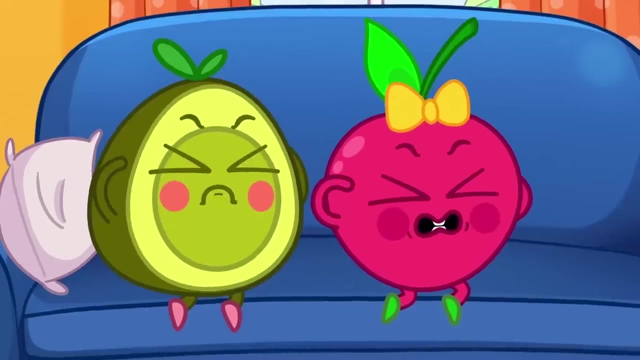 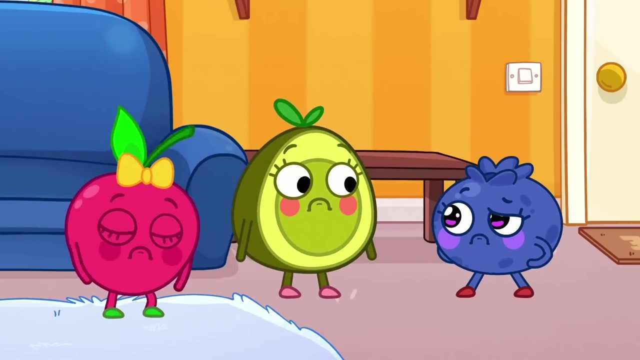 You should always fix what you break. Don't touch toys without asking. If you're hungry, just ask. Oh no, Blueberry has a question. Can I have some food? Of course, Boring Blueberry loves loud music. Not everyone likes loud music. 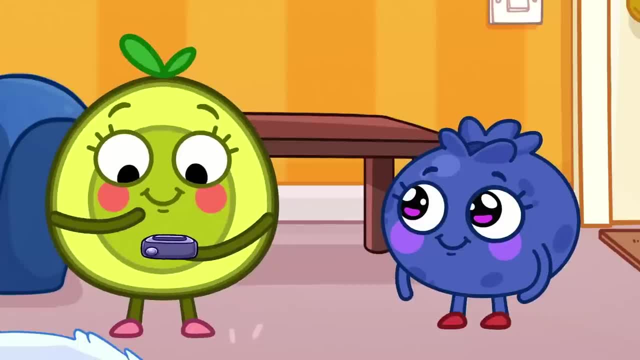 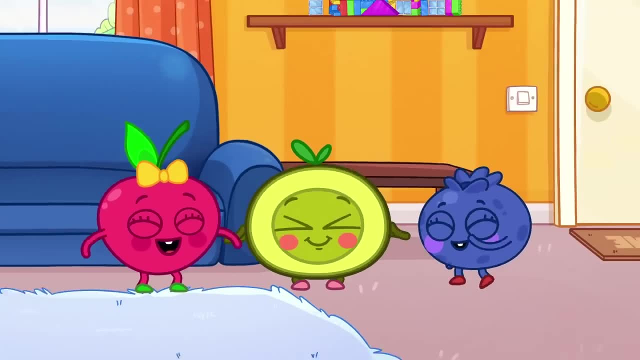 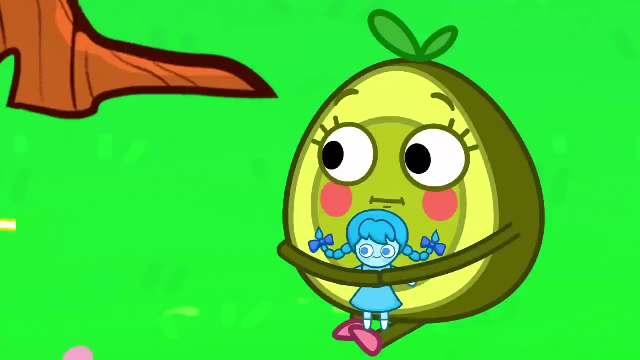 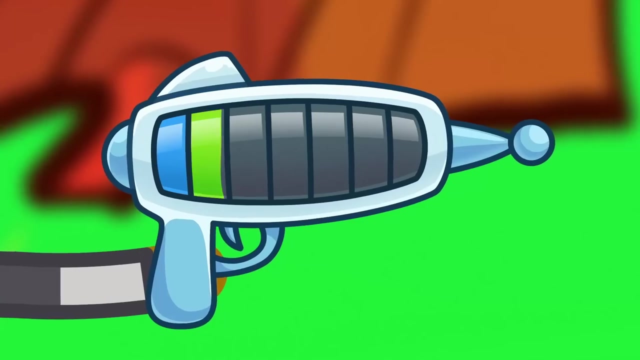 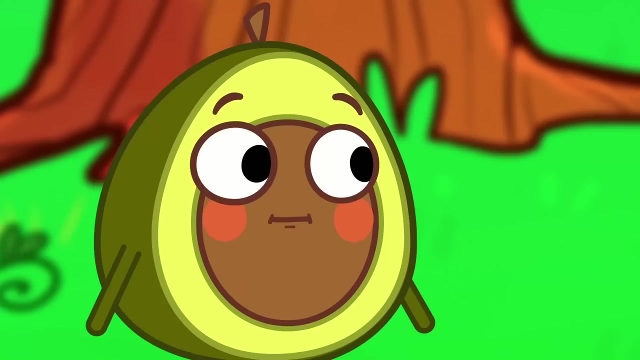 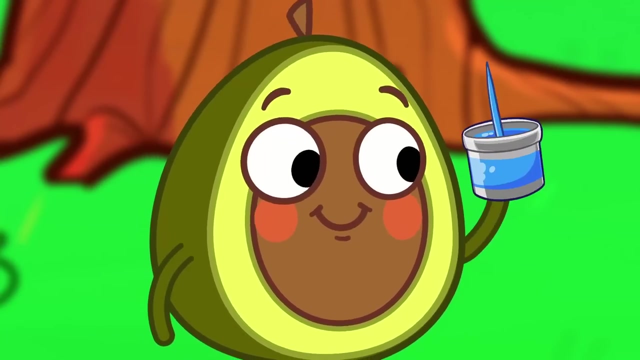 I'm sorry. Find something everyone enjoys. Do you like this music? Have fun, kids. It's Mr Lemon And he's stealing colors. He even stole Penny's green color. Tell Pit what happened. My color was stolen. Maybe Pit can paint on new color. 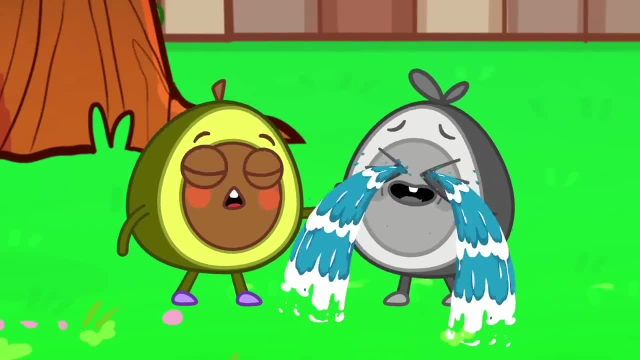 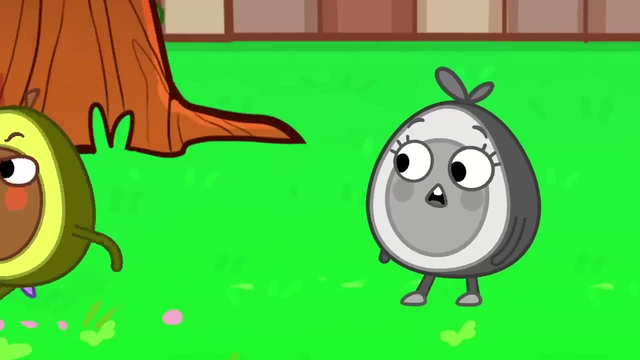 That won't work. We will catch the only two colors. Oh no, Penny's yellow. Have fun with us, And you too. Bother, Bother, Bother. Mr Lemon, There he is again. We will catch the beef of colors. 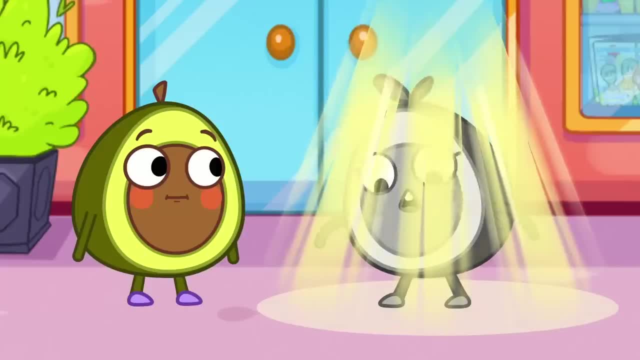 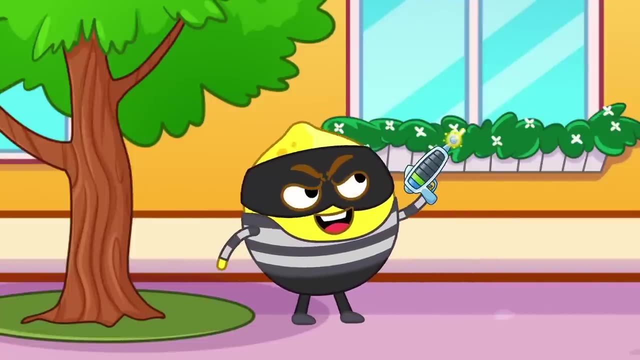 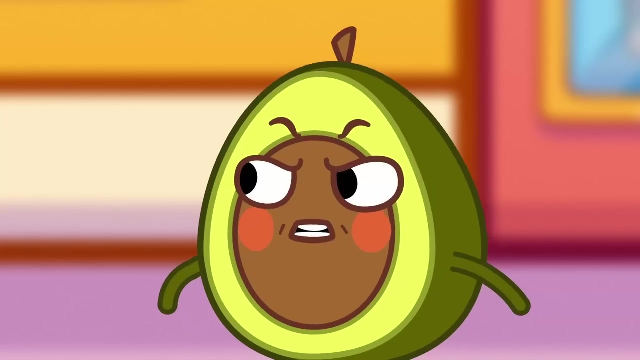 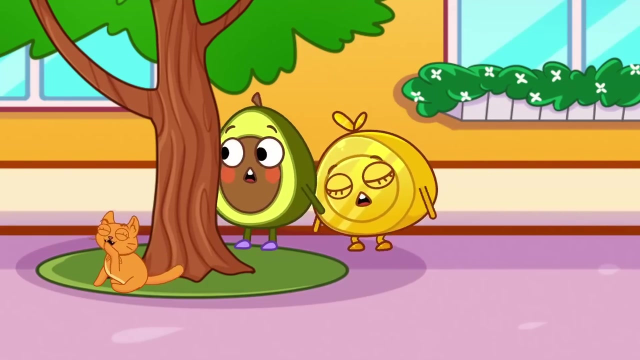 Where could Mr Lemon be? Hello Sun. Now Penny is Golden yellow. Oh no, He stole the Sun's yellow color. Oh no, Oh no, He stole the Sun's yellow color. Oh no, Be careful, Pit and Penny. 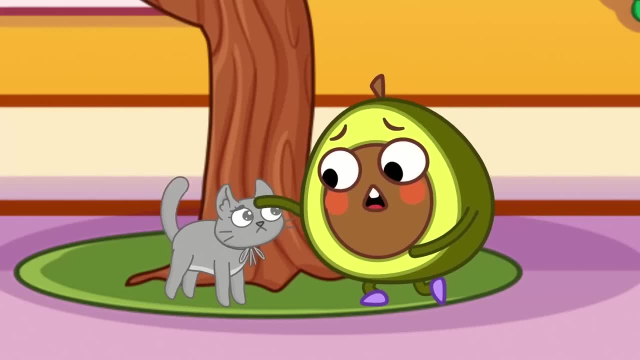 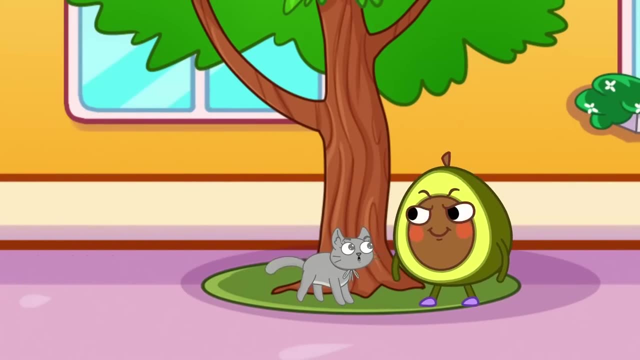 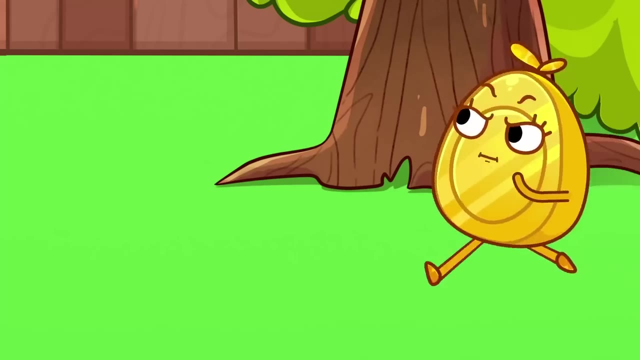 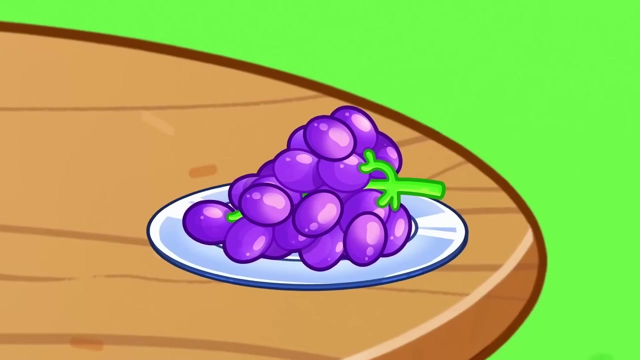 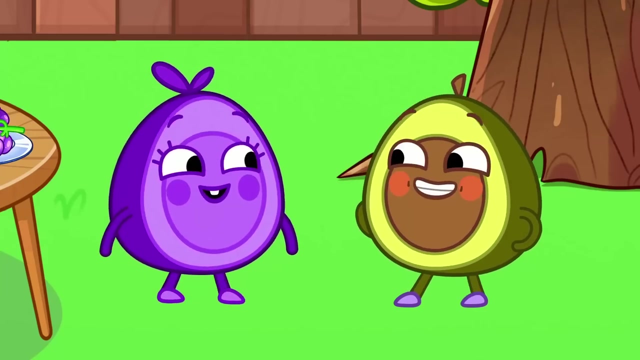 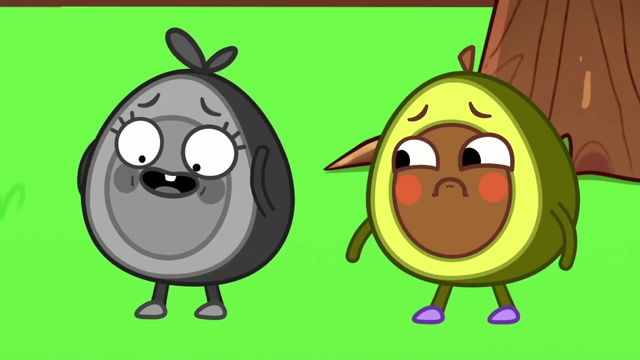 He took the kitty's orange color. I'll get your color back. Come on, Pit, Look. Yummy purple grapes. They turned penny purple. I'm so happy, I'm so happy, I'm so happy. But Mr Lemon took the purple with his ray gun. 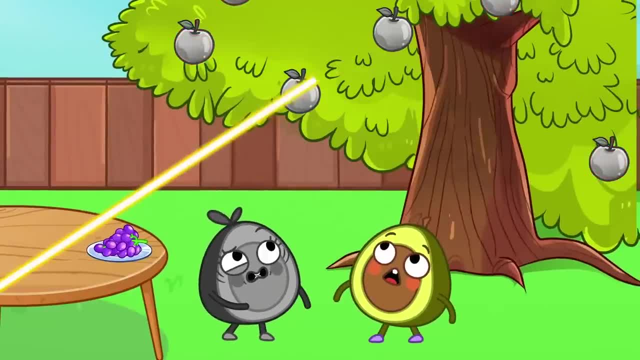 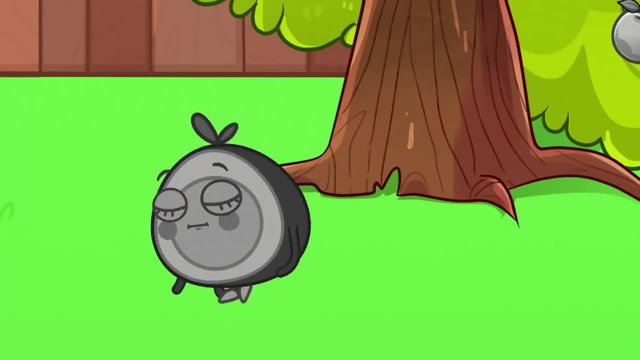 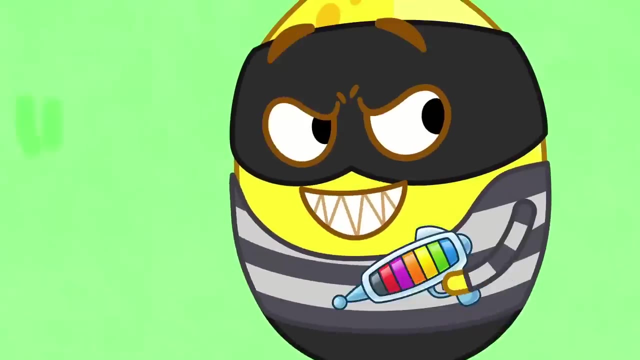 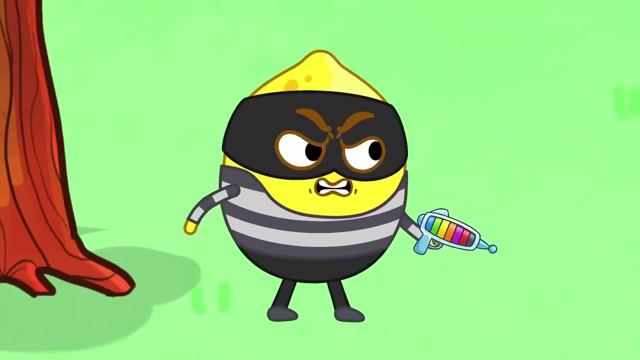 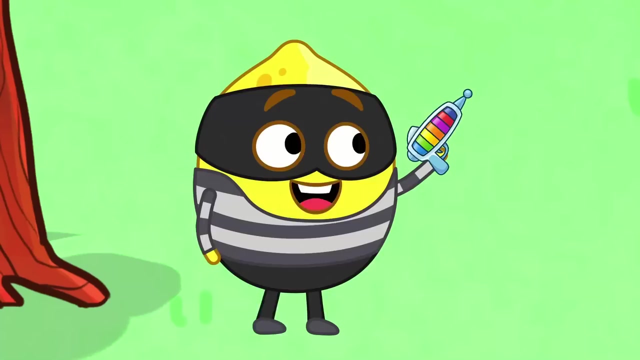 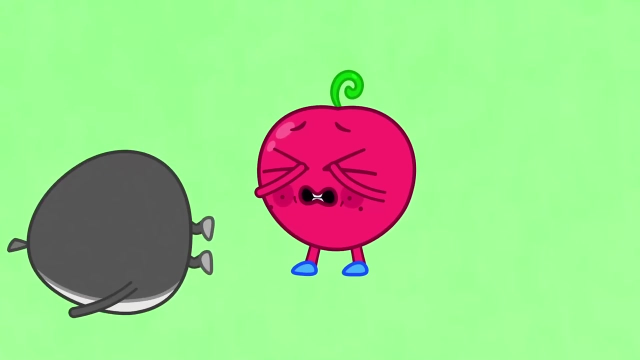 Look, Red apples: Mr Lemon stole the red color Quick, Before he steals any more colors. Watch out Blueberry: Mr Lemon has all the colors now, Poor Pit. Now Mr Lemon has too much color, Phew. 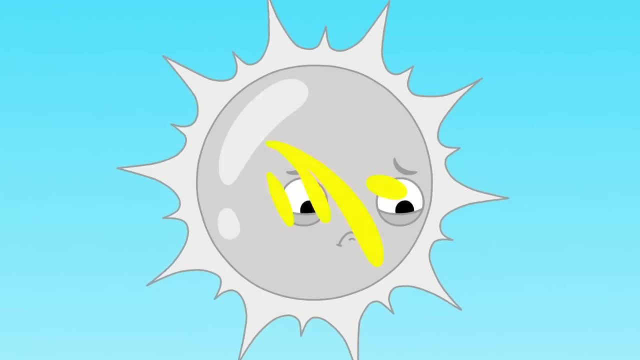 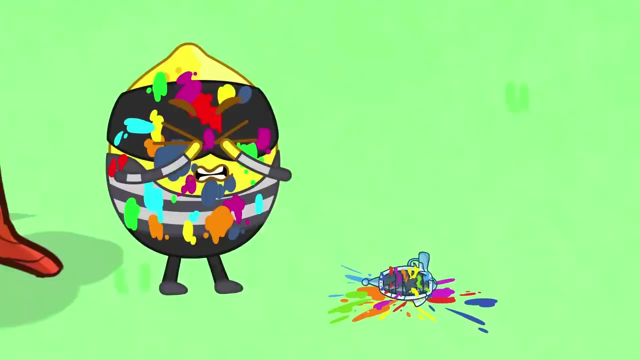 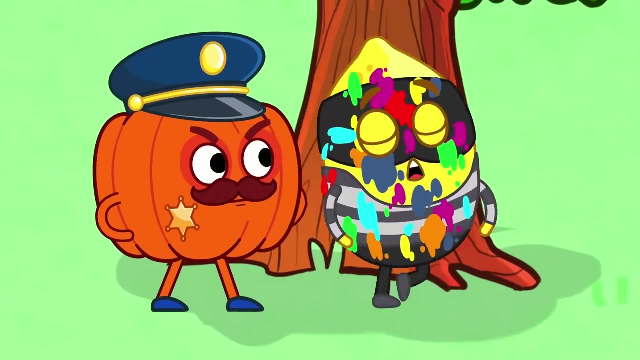 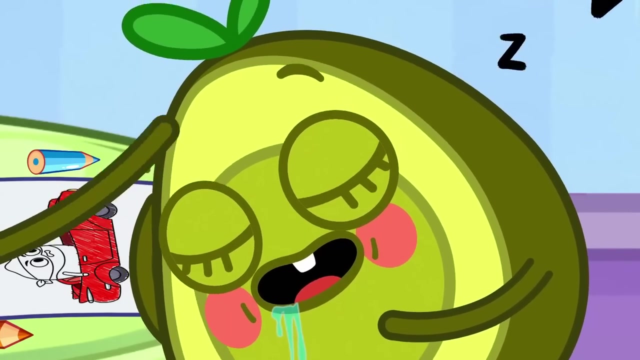 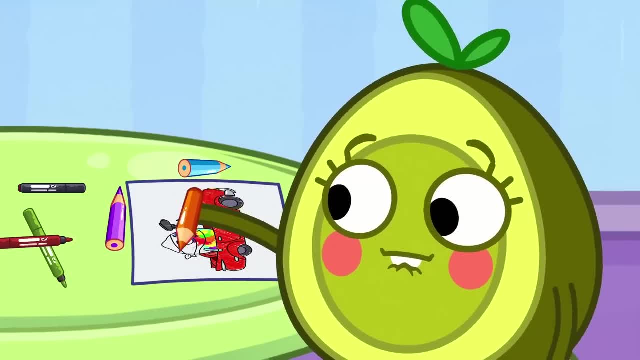 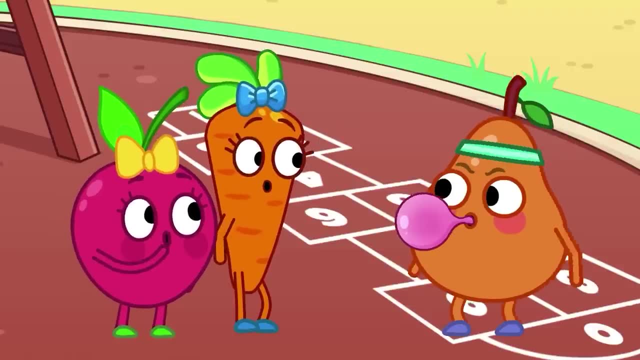 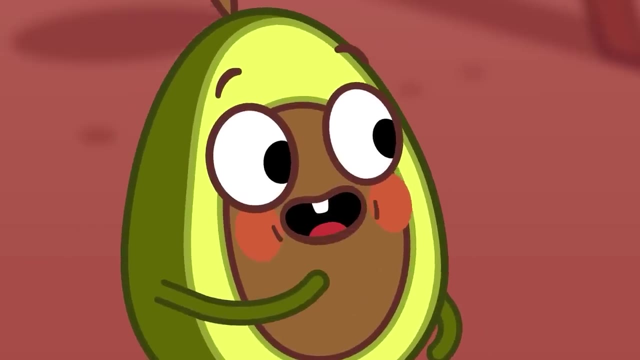 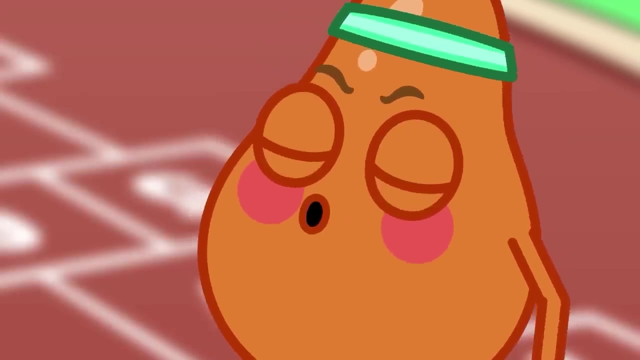 What color will you use, Penny? All of them, of course, All of them, of course. Piercy is blowing a bubble. Oops, This bubble popped. Look at me, Can Pit blow a bigger bubble? Piercy wants another try. 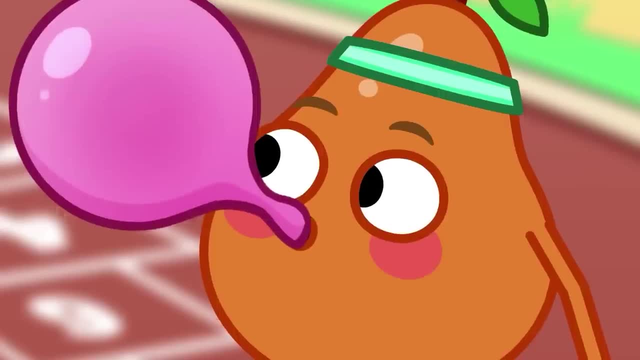 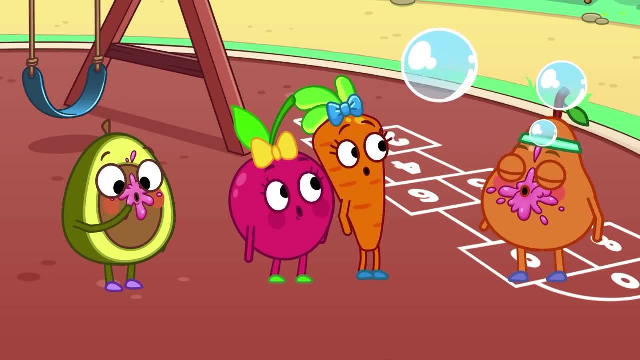 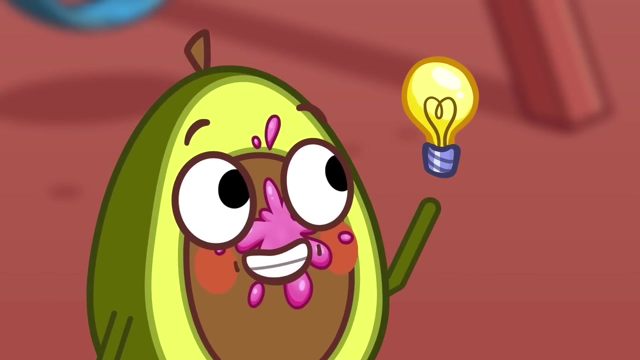 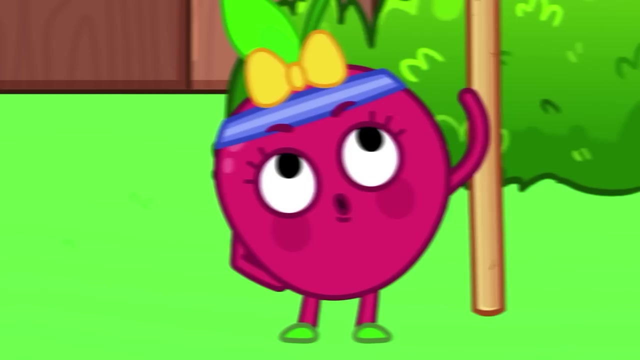 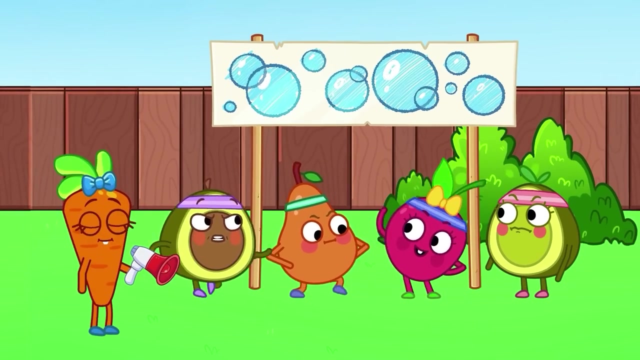 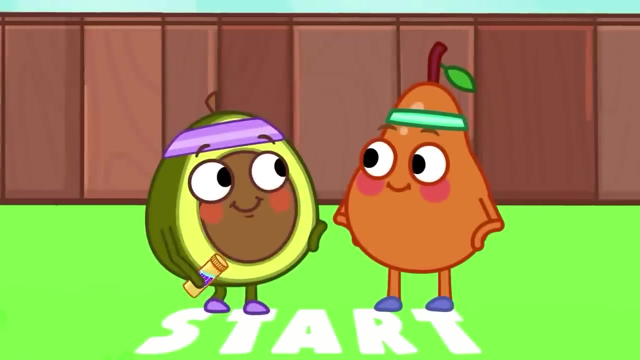 Look, An even bigger bubble. Where are these bubbles coming from? Penny's making them. Pit has an idea. The kids are going to have a bubble-blowing contest. Here comes the judge. Start the competition. Pit's up first. 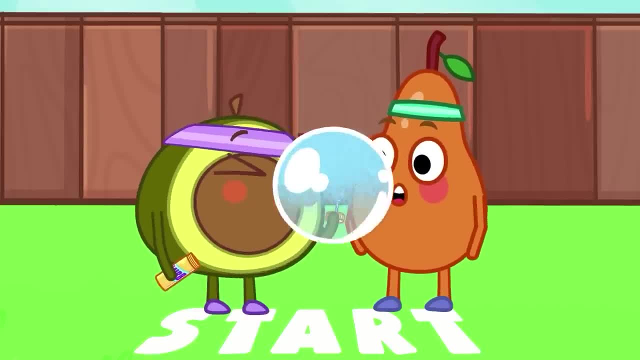 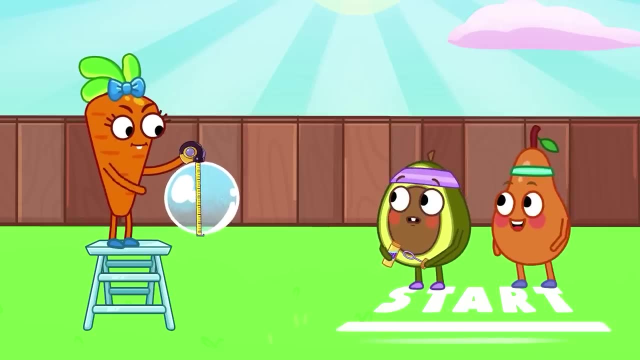 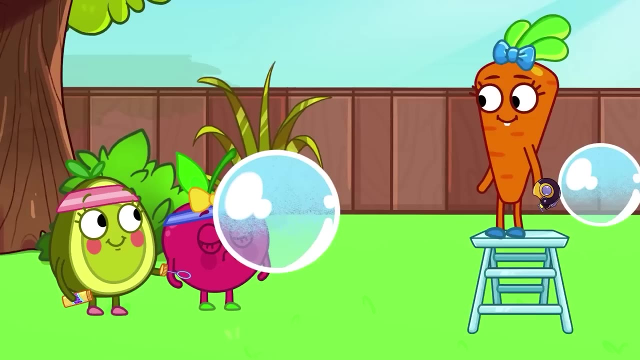 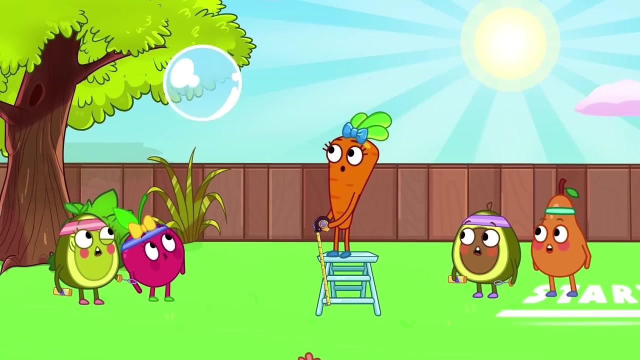 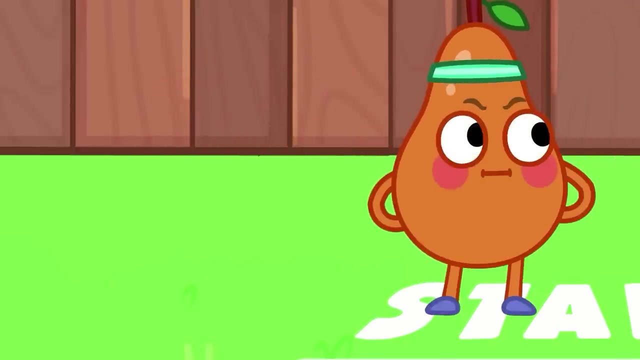 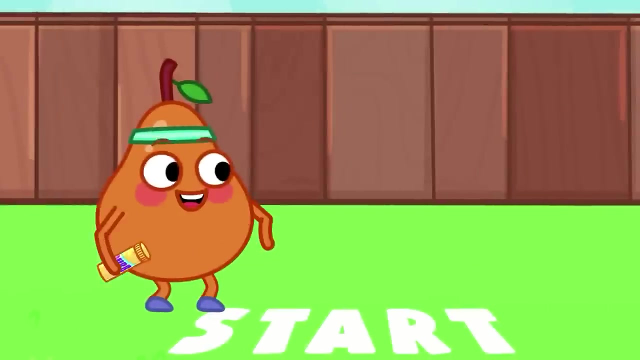 Good luck, Pit. Not bad Your turn, Penny. Good luck. Be careful, Carrot. Looks like Penny is in the lead. Huh. But Pit has a plan: He'll use the leaf blower. Will it work? 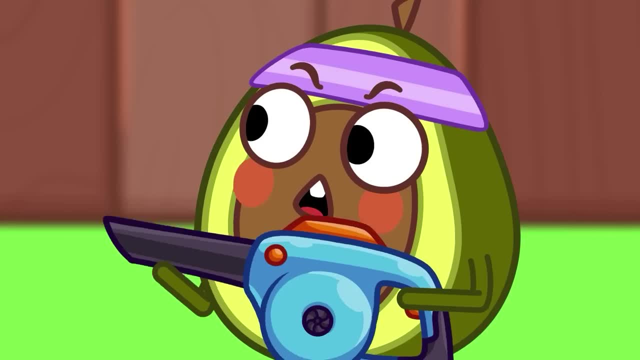 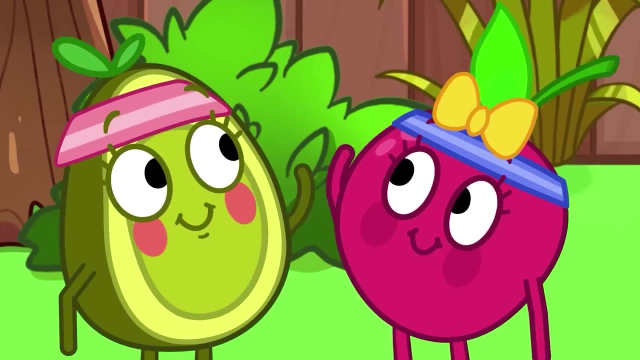 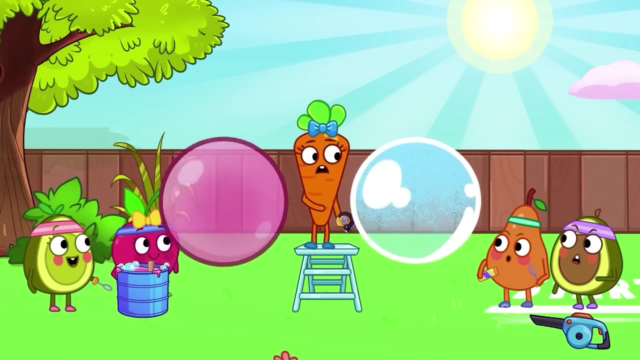 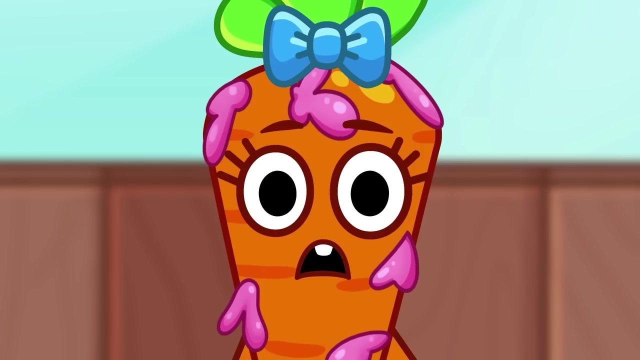 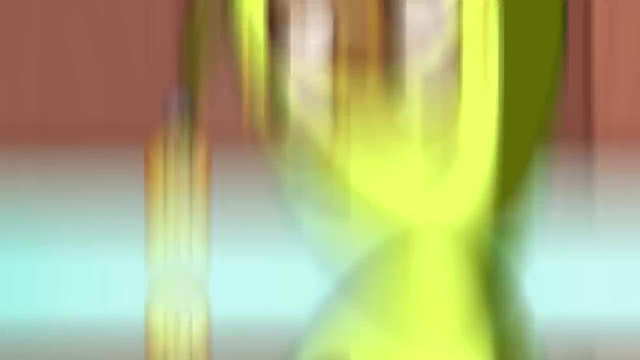 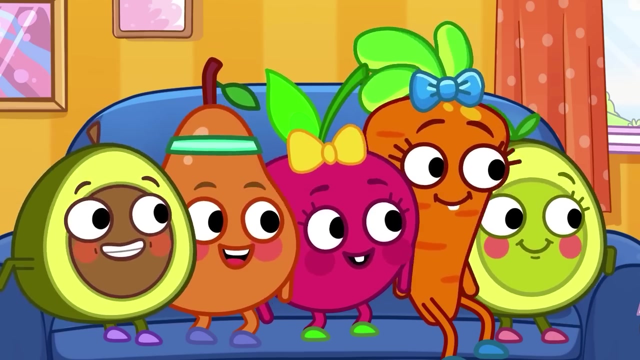 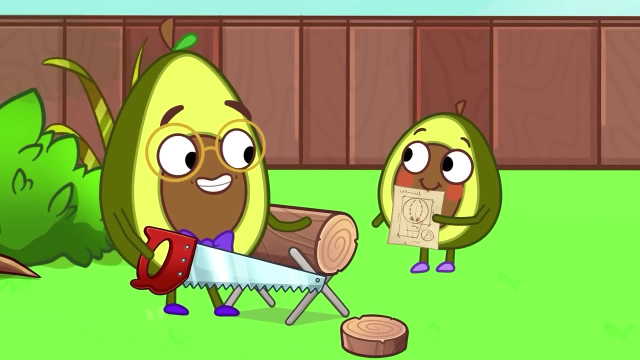 It did. That bubble is huge. Cherry wants to mix a soap bubble and bubble gum. He's so cool. will this work? oh no, look at this mess. maybe daddy can help kids. let's build an air balloon together. daddy will cut the wood, penny will make the basket. 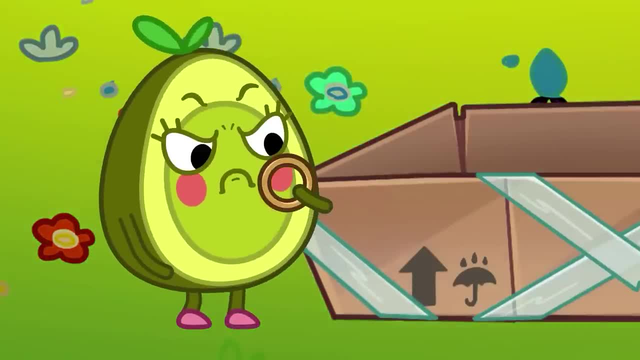 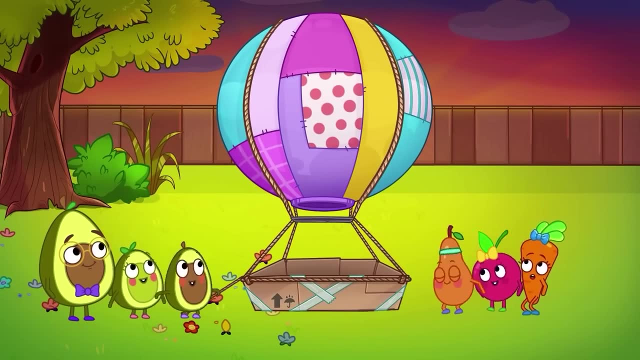 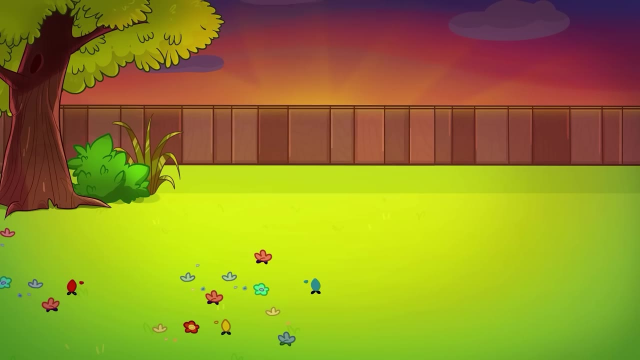 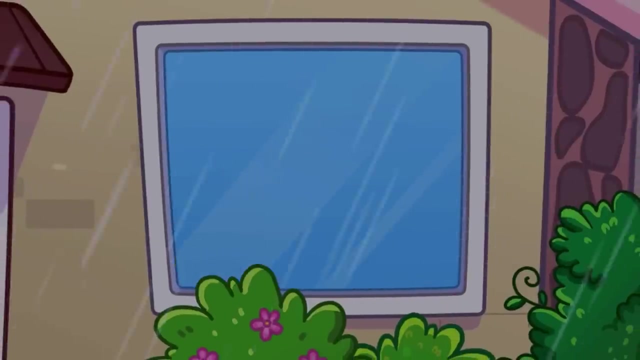 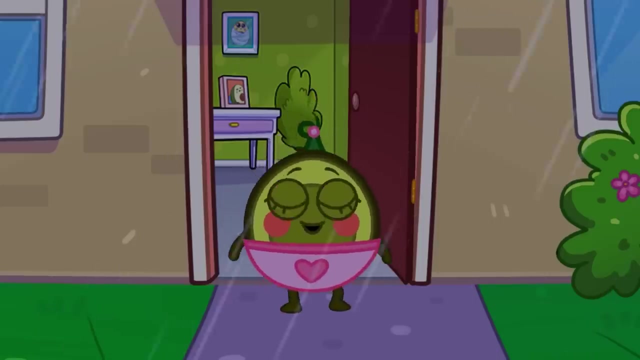 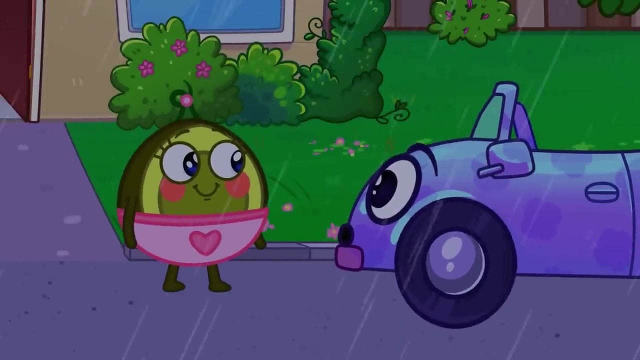 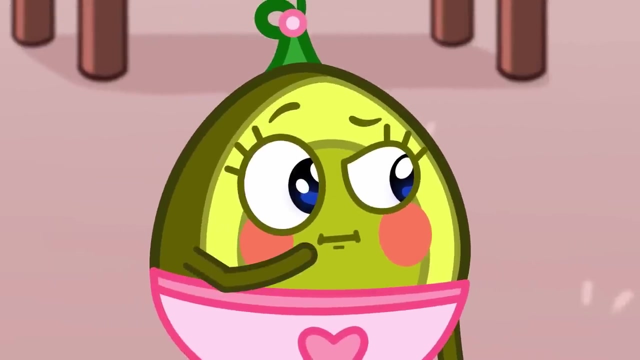 here. see to the rescue. everyone in an air balloon is like a bubble that won't pop. have a safe flight. you toy car is scared and alone outside. who's that? it's baby and she wants to play. toy car has mud on him. baby has an idea. 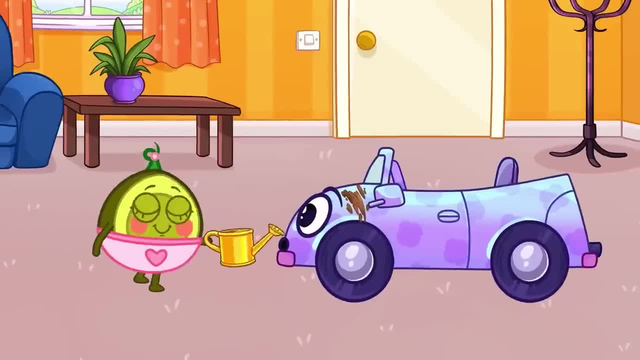 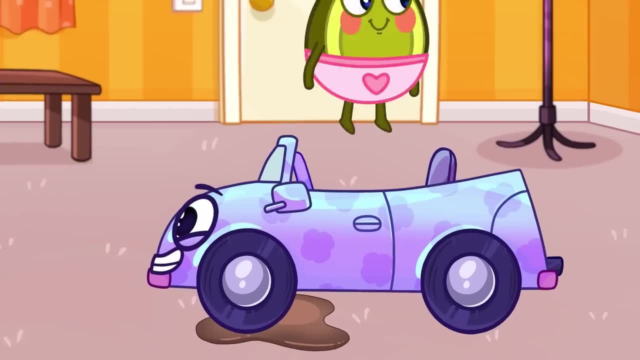 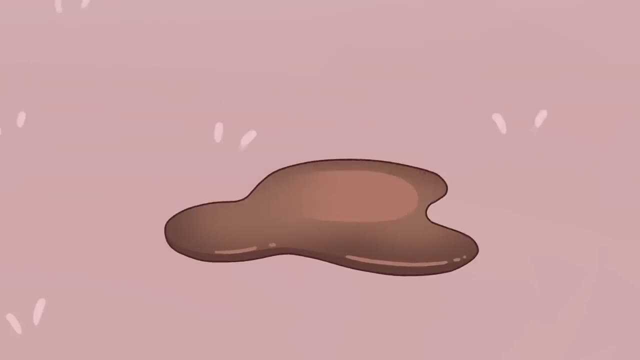 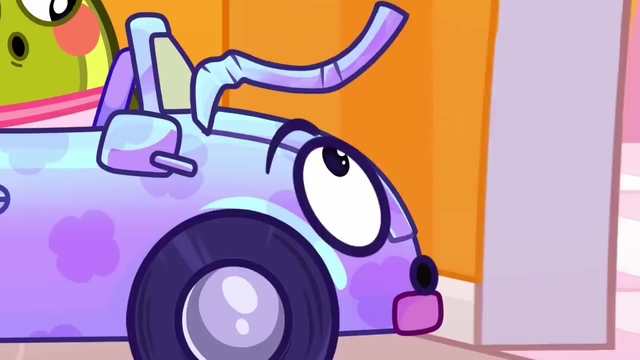 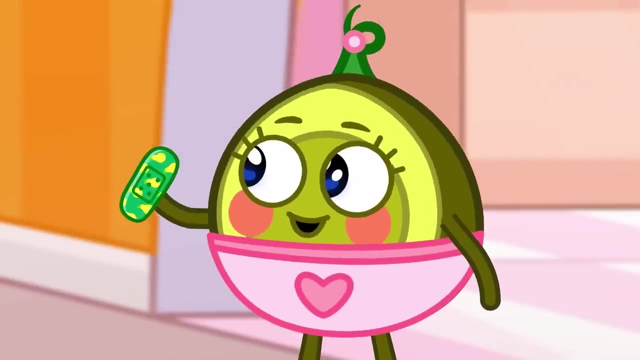 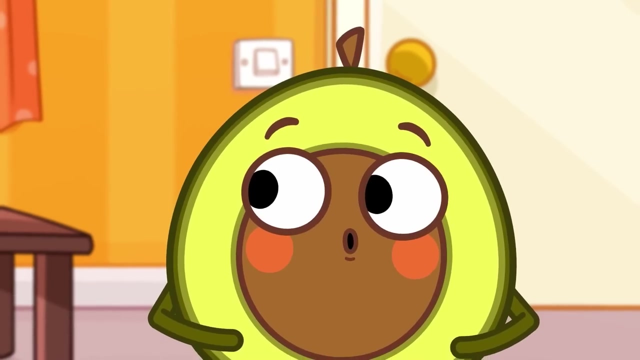 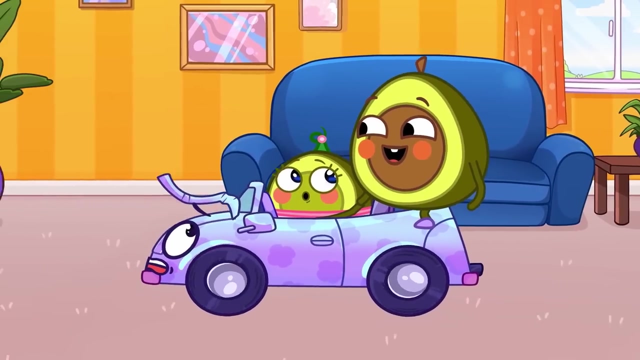 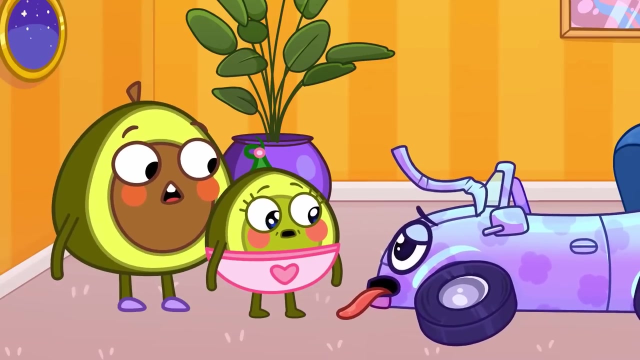 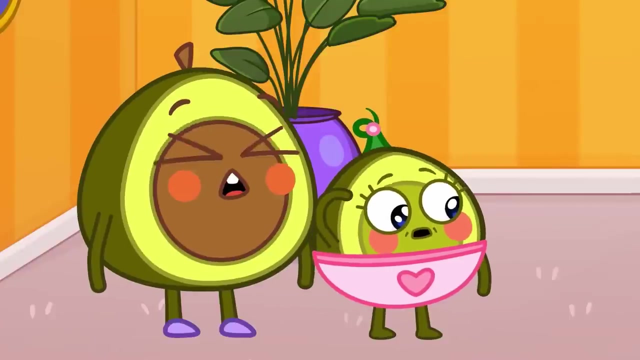 now toy car is all clean. oh no, there's been an accident. baby knows what to do. oh no, here's a bandage for your boo-boo. i want to play too, kid, you're too big. toy car has run out of energy. oh oh oh, baby wants to feed it milk. 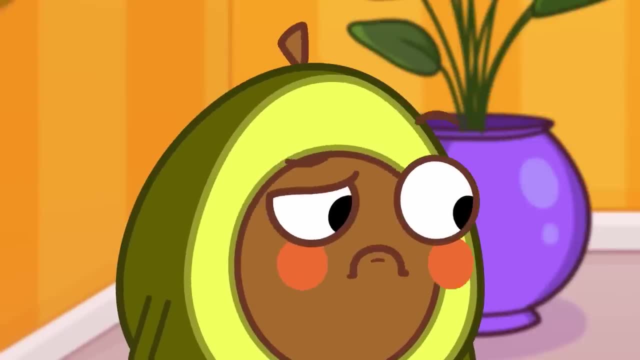 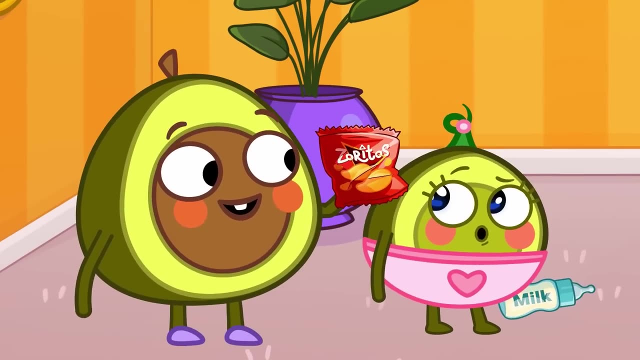 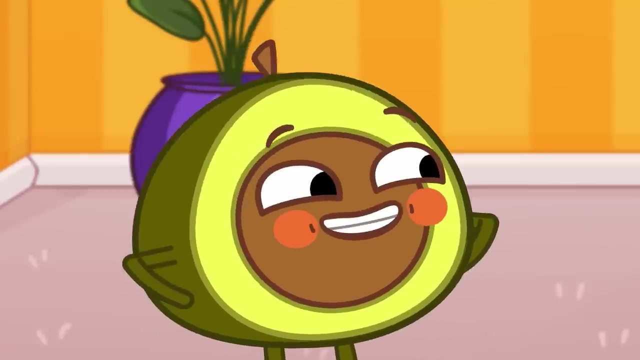 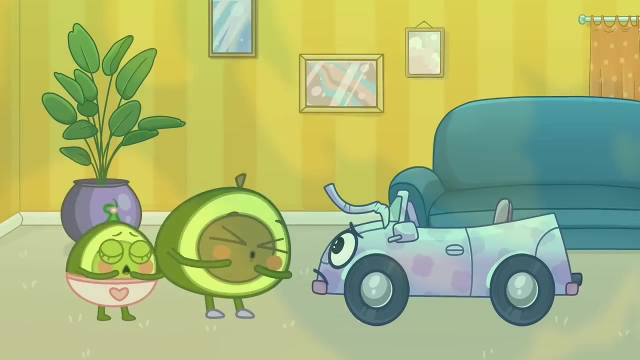 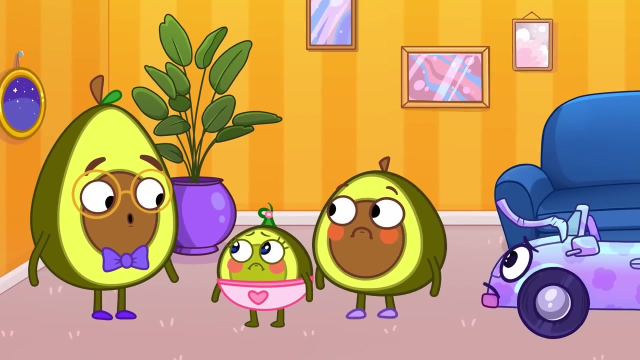 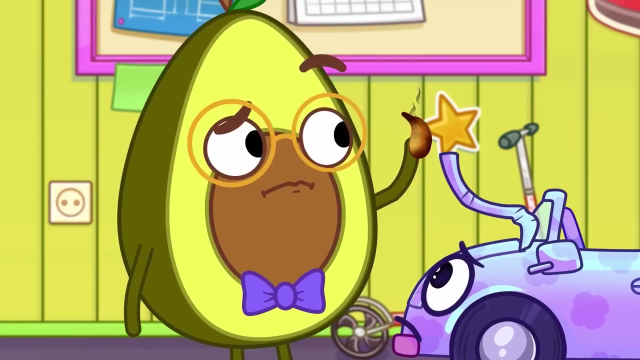 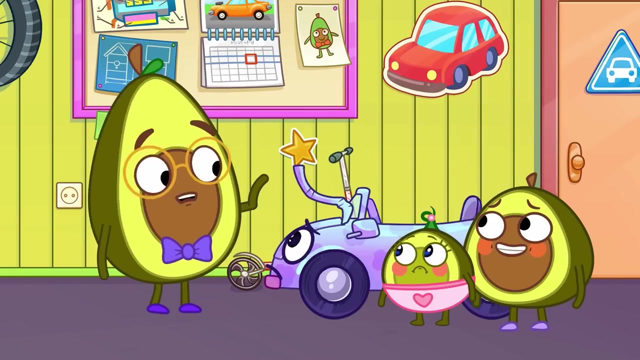 this is for little babies. oh pit, wants to feed toy car some chips, but chips aren't for cars. some toy car's aren't for cars. some toy car's aren't for cars. Maybe daddy can help. Each toy needs proper care. Toy car runs on electricity. 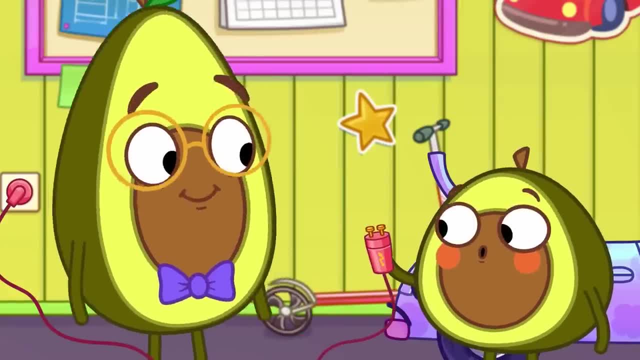 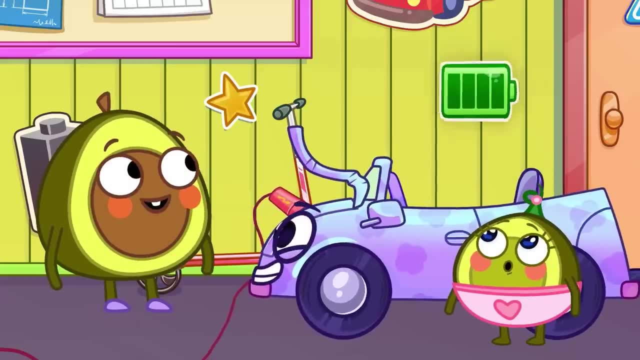 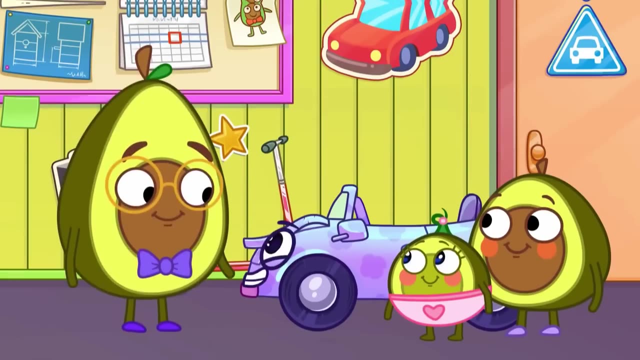 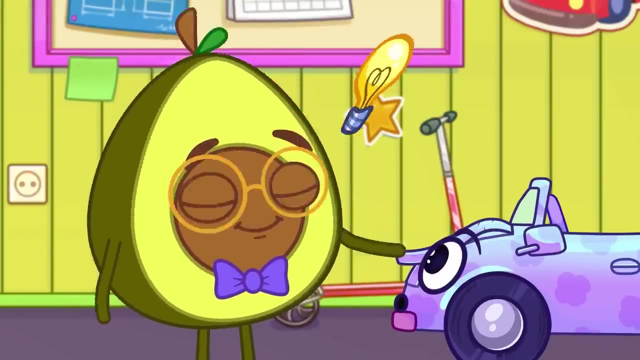 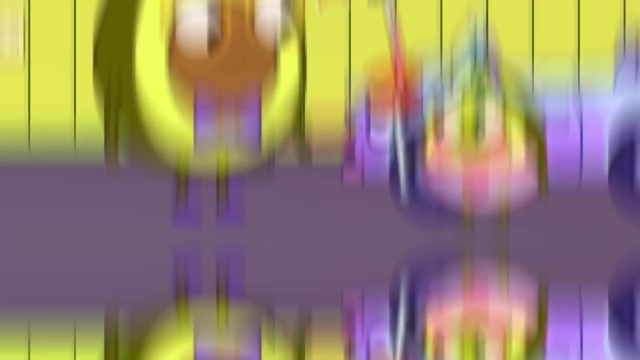 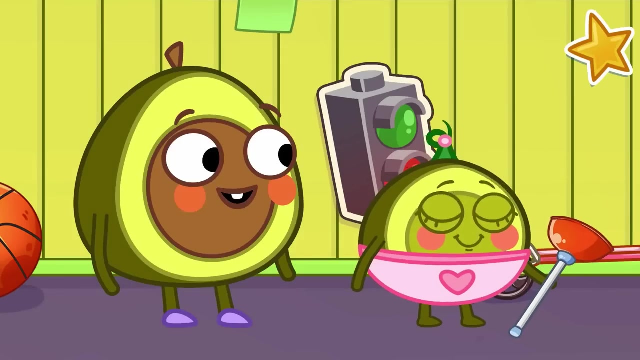 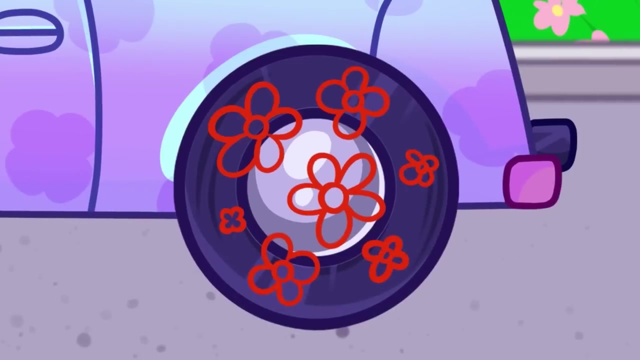 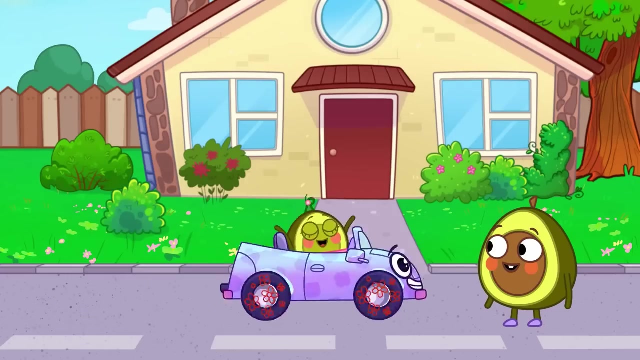 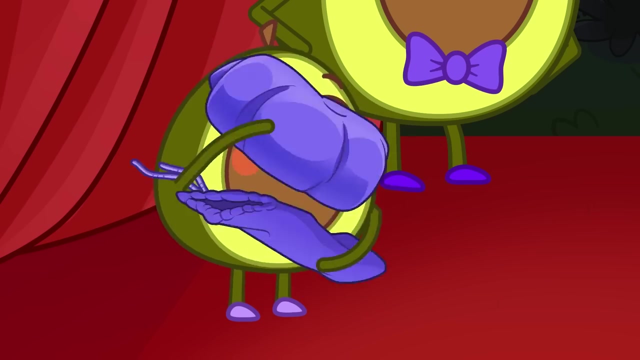 You must plug it in for energy. It worked, But the hood is still dented. A plunger can help with that. That's better. Hop in. baby Toy car is ready to play again. Pit and Penny are camping with their family. 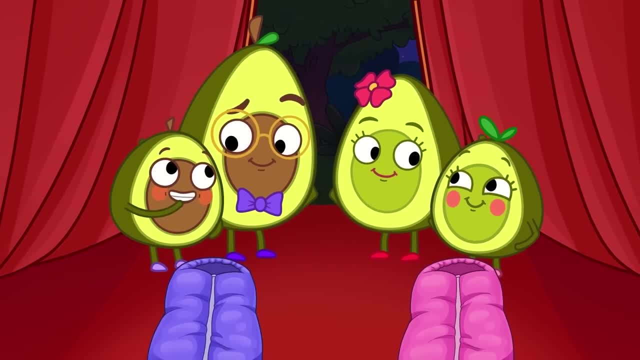 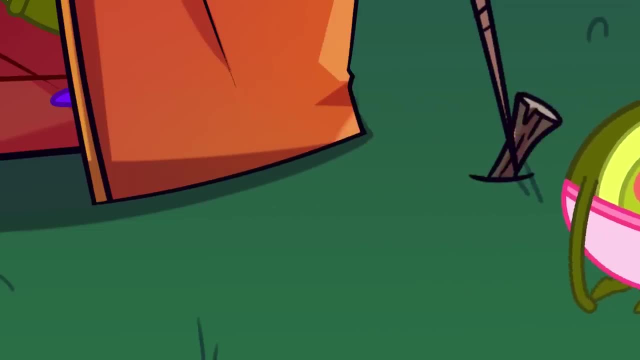 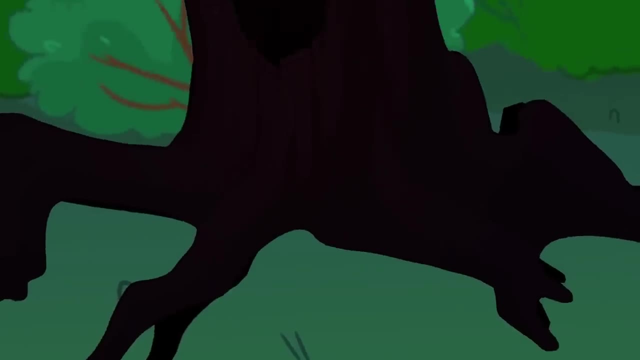 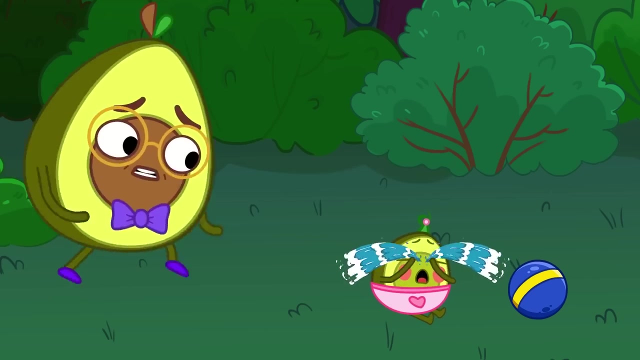 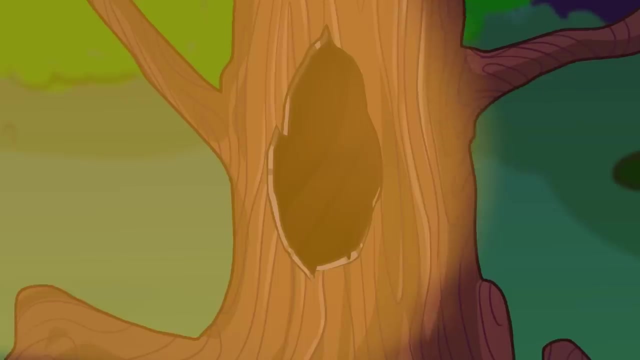 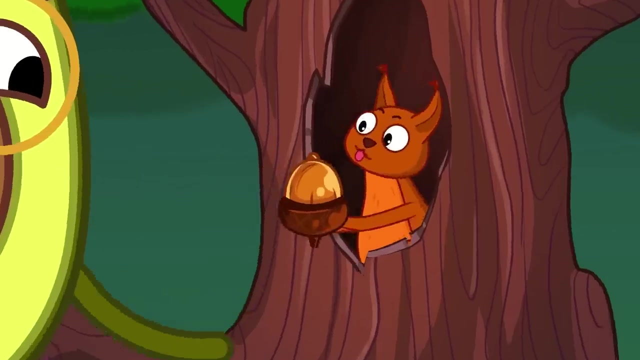 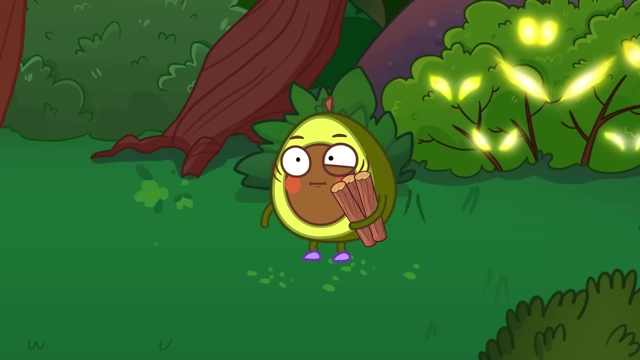 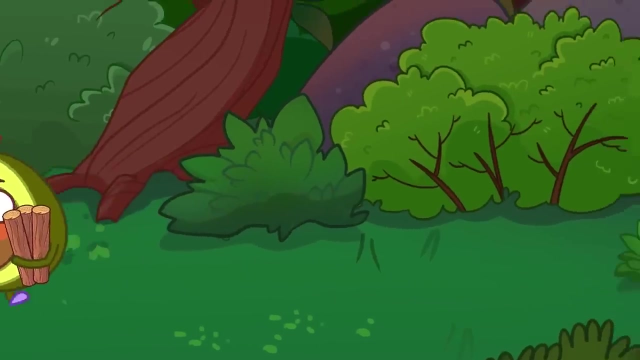 Baby is playing with her ball. Oh no, Her ball rolled away. Is that a monster in the woods? Daddy, Baby saw a monster. Phew, It's just a squirrel in a tree Pit is collecting firewood. Something's in the bushes. 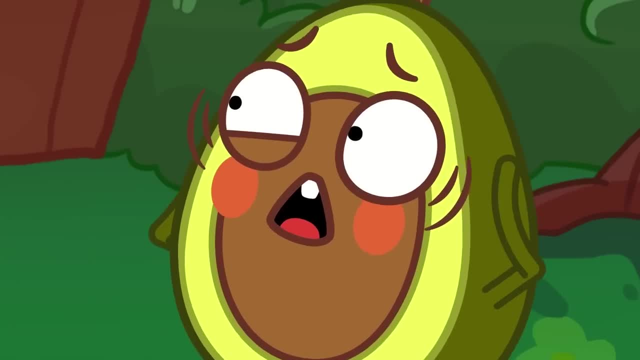 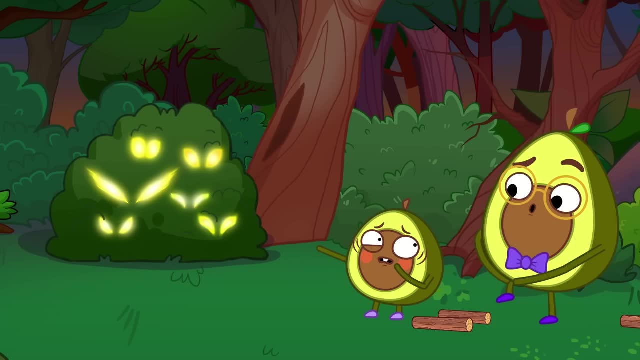 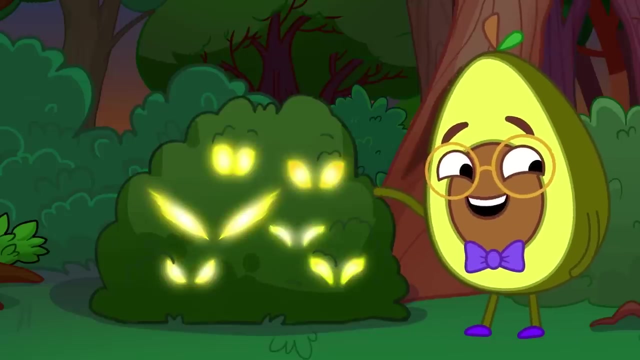 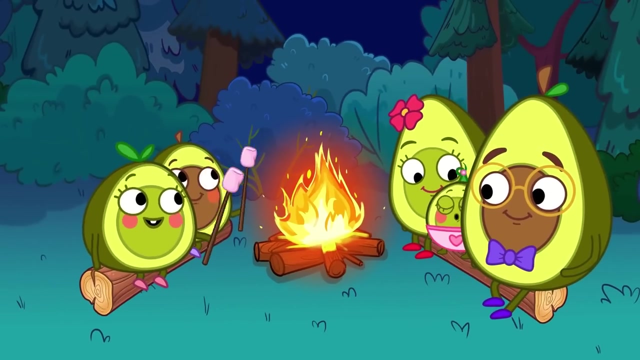 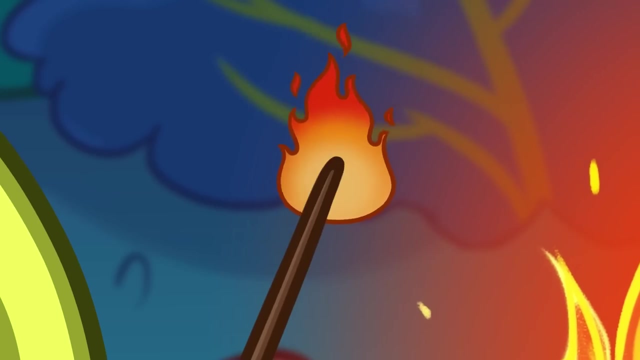 What could they be? They're a monster. What's so funny, daddy? These are fireflies. The family is roasting marshmallows- Yum Oops, Penny burnt that one. There are more marshmallows by the tent. 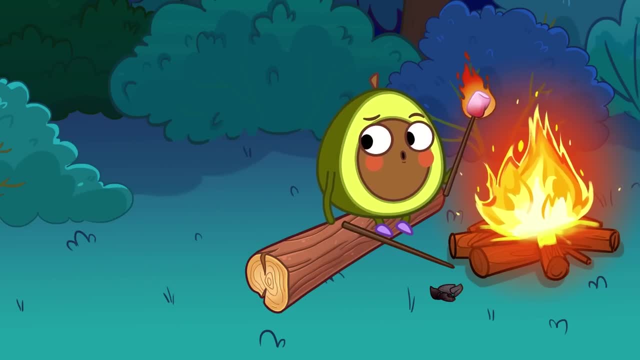 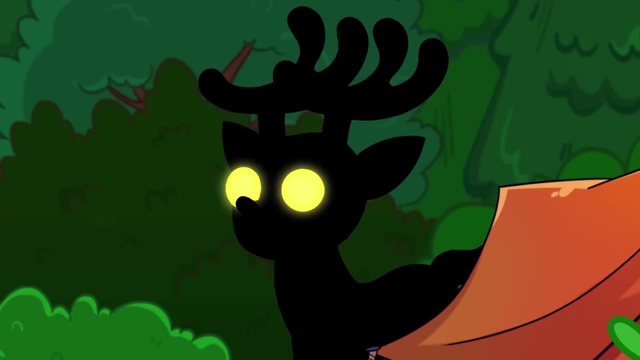 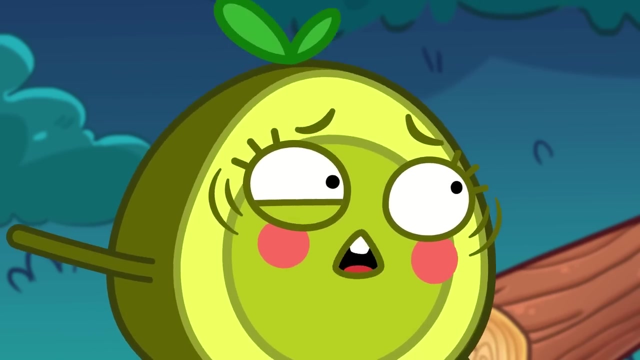 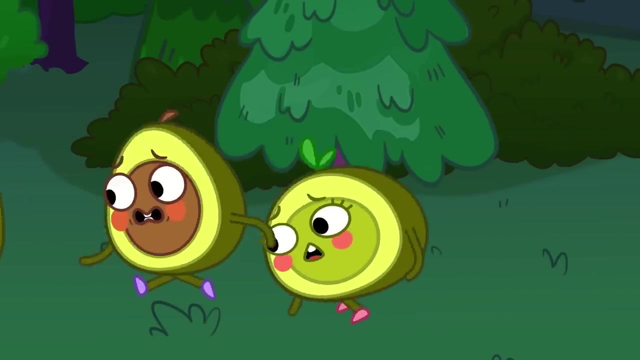 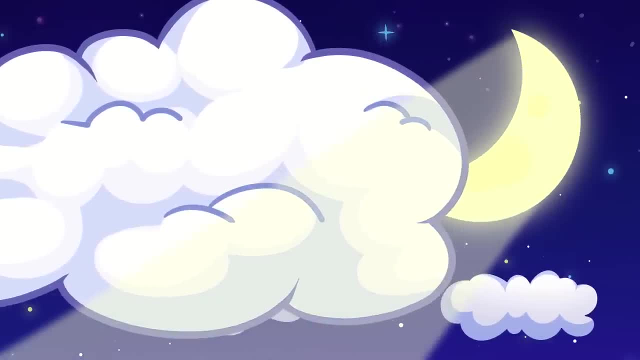 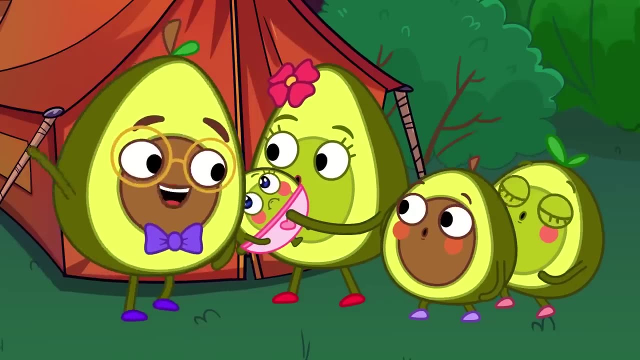 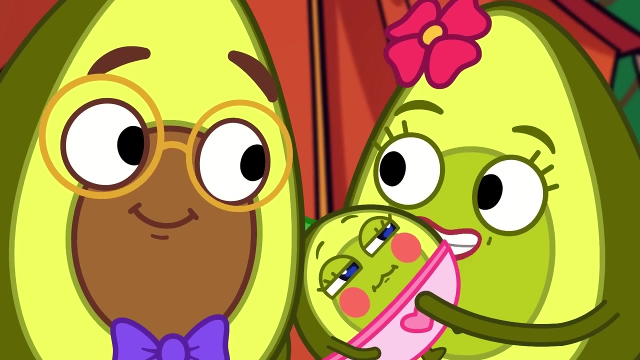 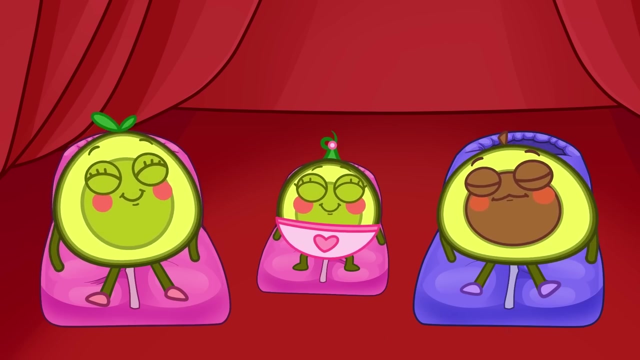 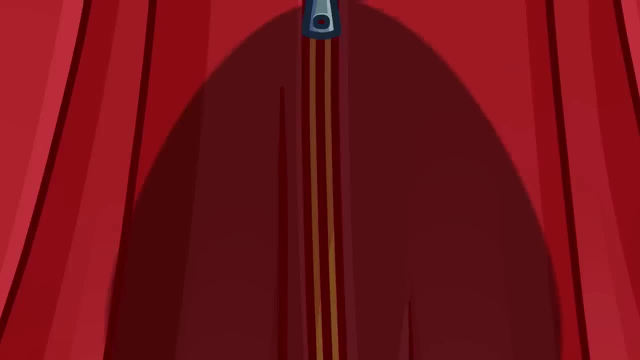 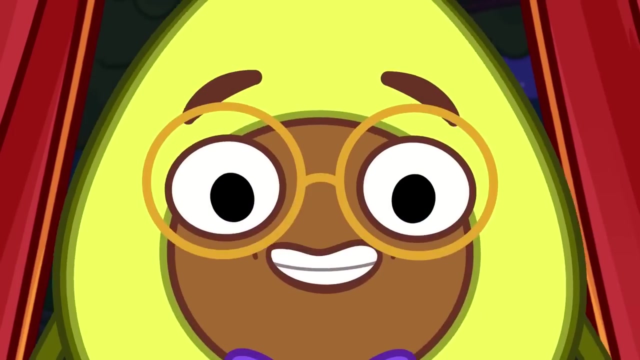 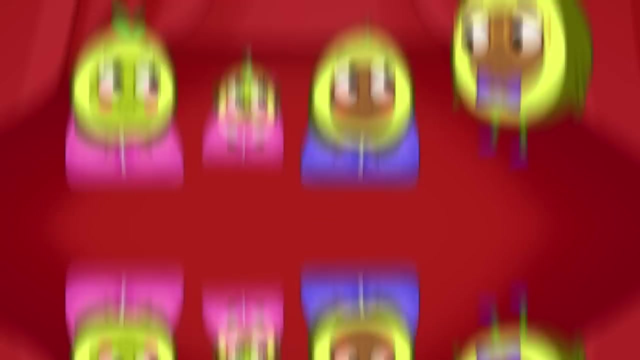 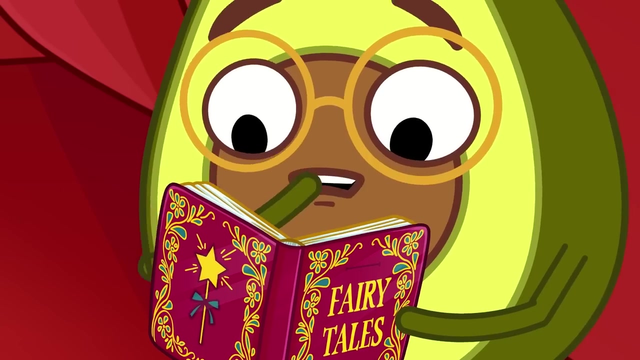 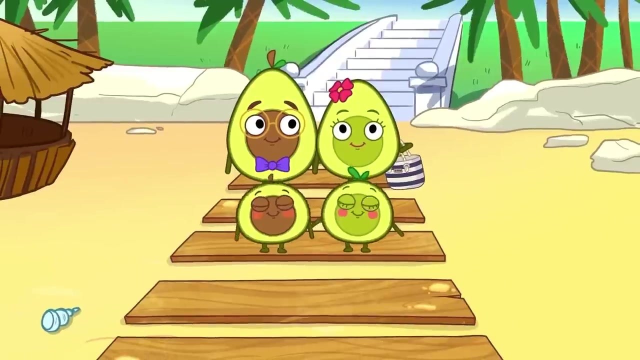 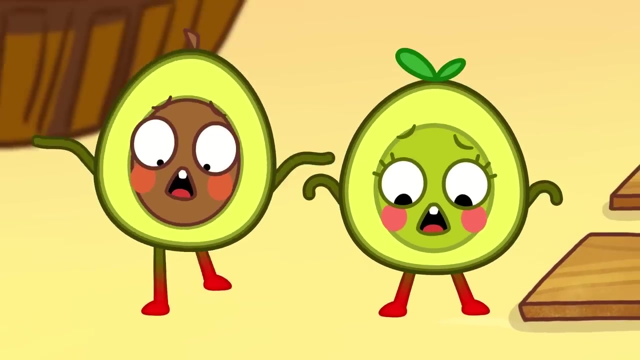 And it's opening the zipper. It's Daddy. We thought you were a monster. Monsters only exist in fairy tales, So there's no reason to be scared. There were three brave avocados. Pit and Penny are at the beach with Mommy and Daddy, But be careful, the sand is very hot. 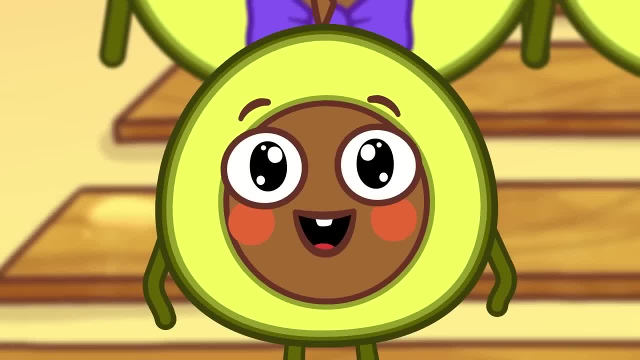 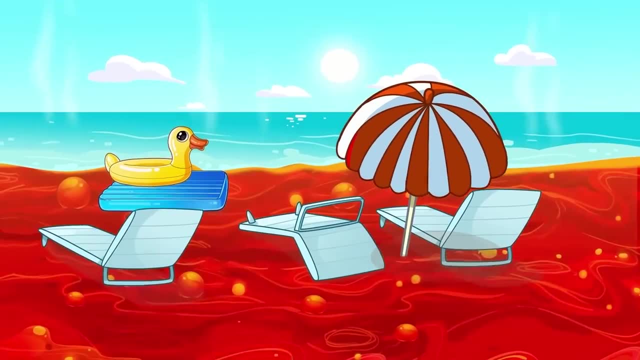 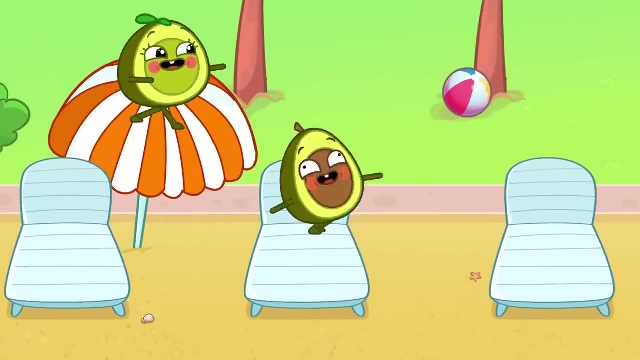 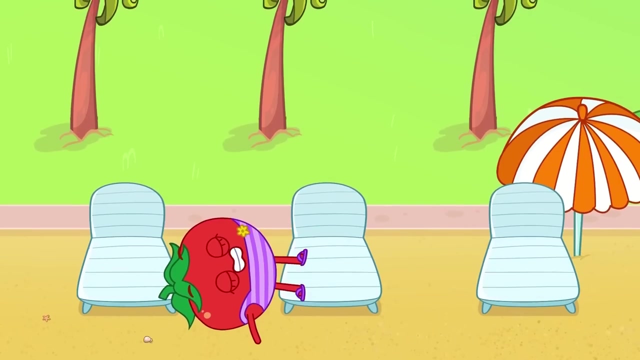 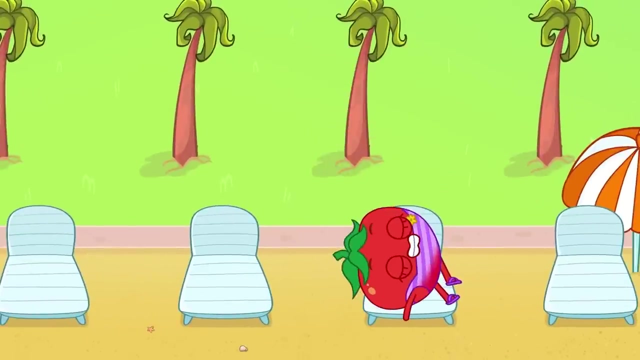 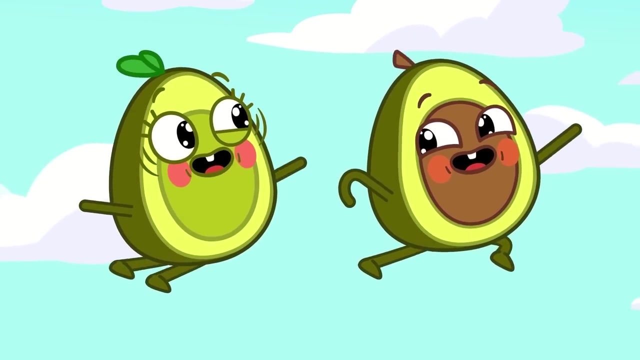 Pit pretends the sand And his lava. He wants Penny to pretend it is lava too. How far can they go without touching the sand? Just watch out for Mrs Tomato. Oh no, Are you okay, Miss Tomato? Will you talk to them? Mommy and Daddy. 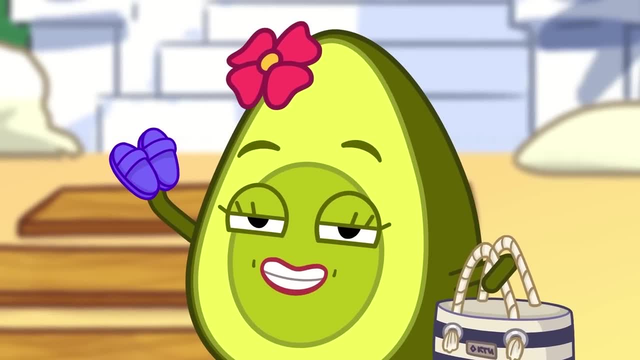 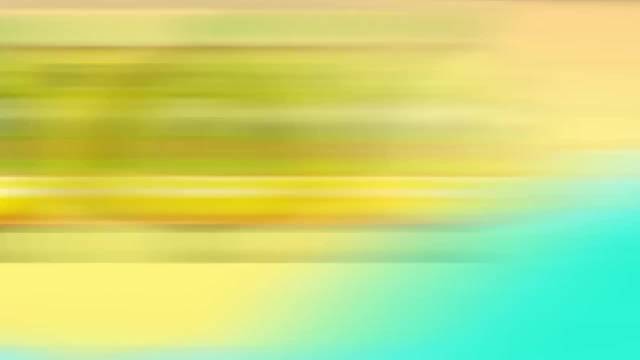 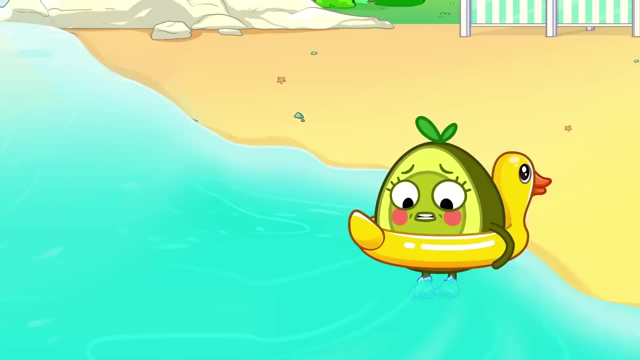 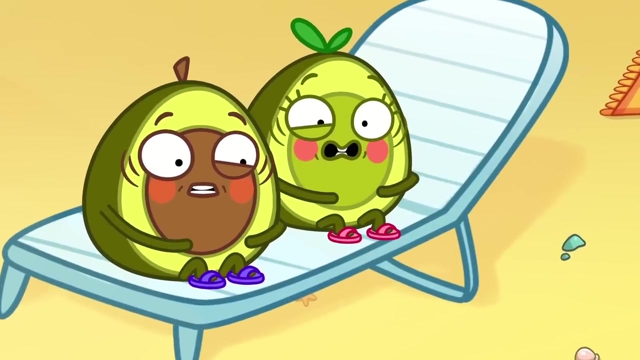 Mommy has an idea: Flip-flops will keep their feet off the hot sand. Penny is ready for a swim, But the water is very cold. But the water is very cold, But the water is very cold. Poor Pit and Penny. But Daddy has nice warm towels for you both. 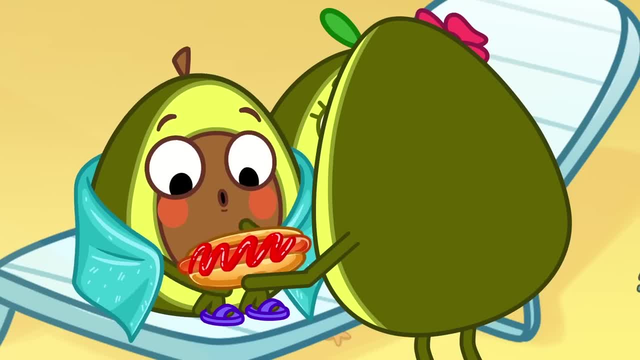 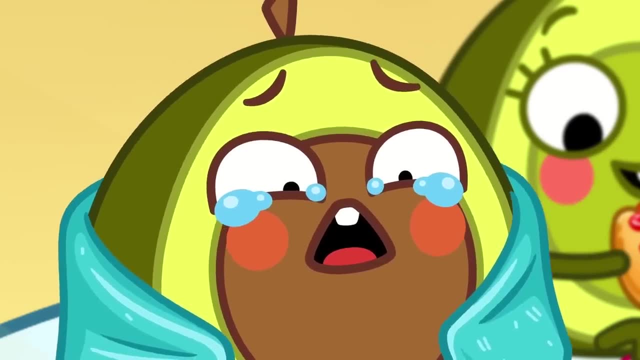 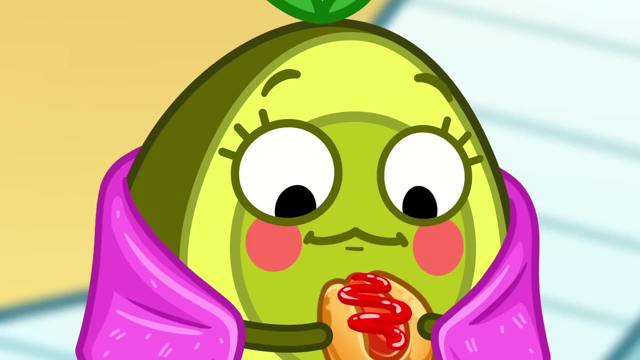 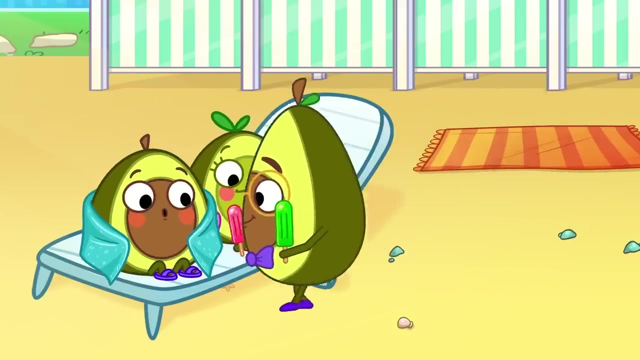 That's much better. Careful Pit that might be too hot. A cold glass of water will help. A cold glass of water will help. A cold glass of water will help Get rich all of you. A cold glass of water will become cold, A nice, clean dish. 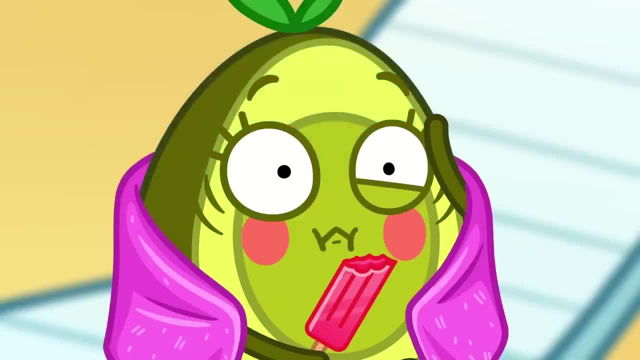 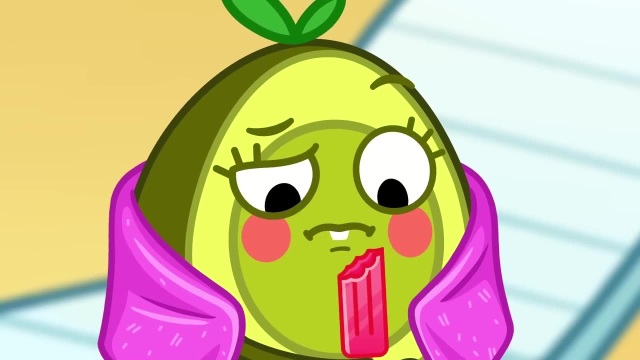 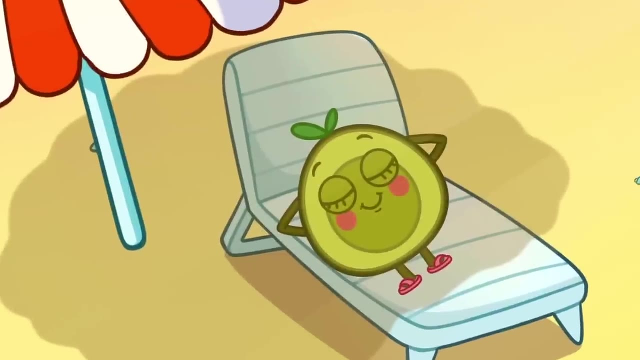 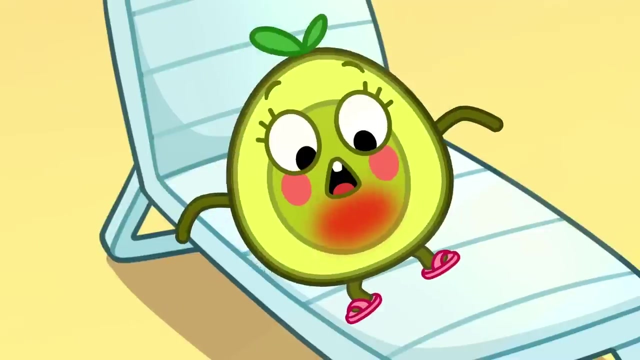 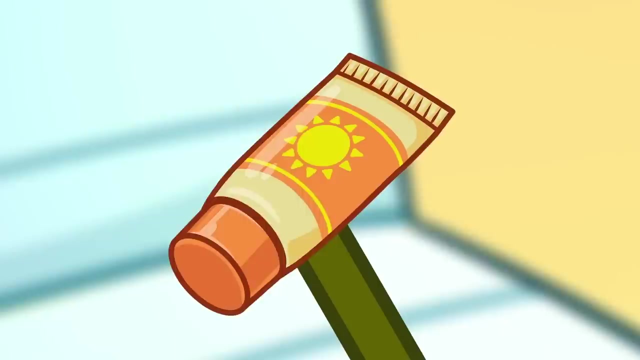 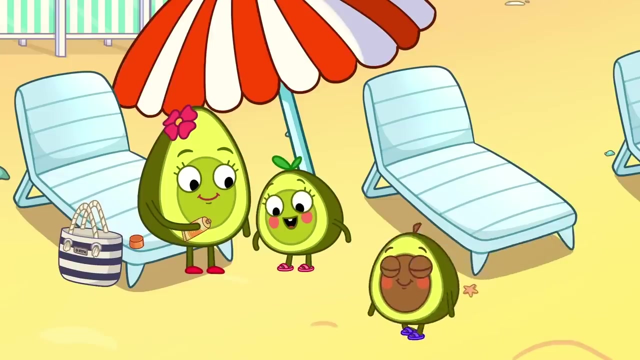 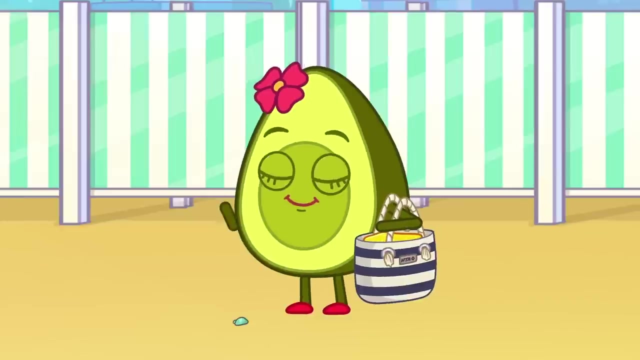 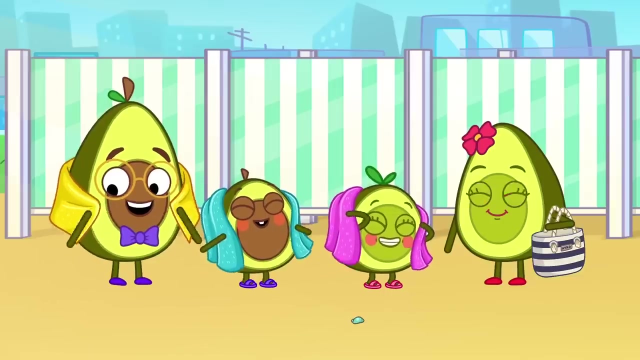 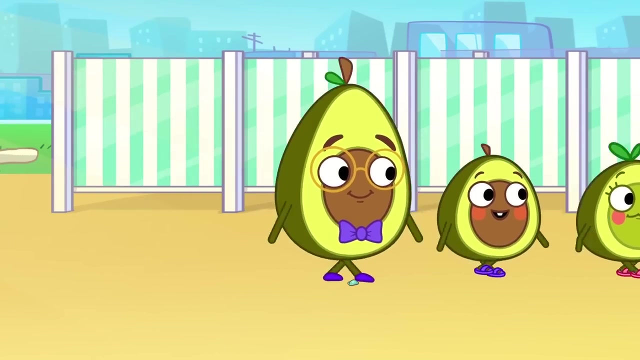 Unties the yogurt Chewing. Penny is resting in the cool shade, But the sun is far too hot. Can Mommy help? Sunscreen will keep Penny safe from the sun. It's time to go home. Bye-bye, Pit Penny, Mommy and Daddy. 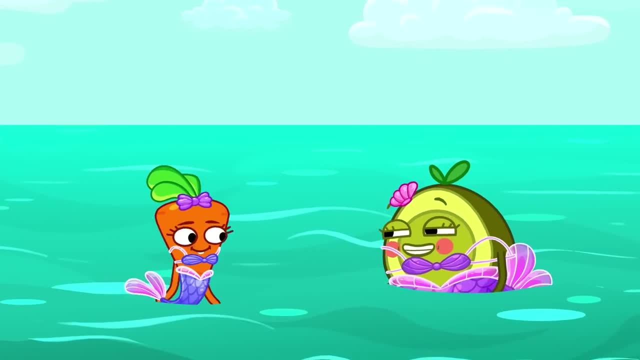 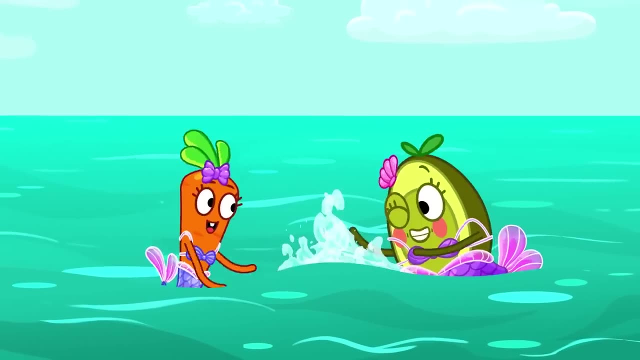 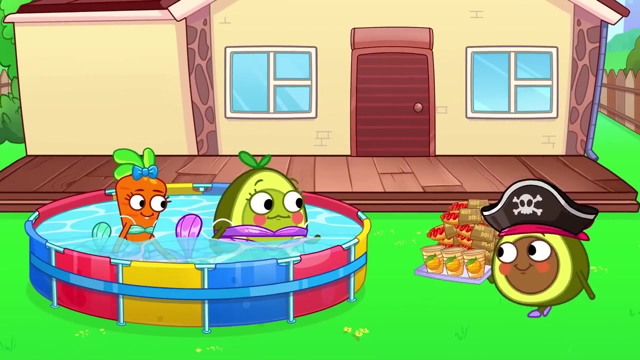 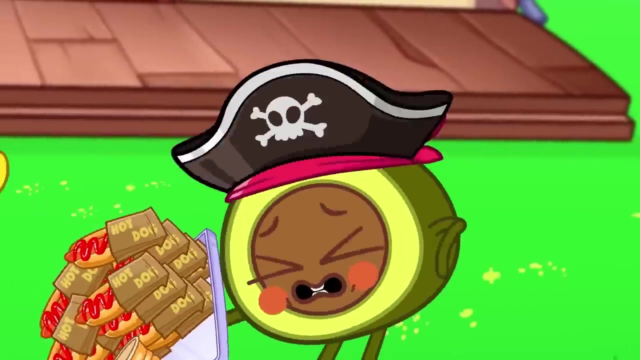 Penny and Carrot are mermaids. It's fun playing in the ocean, Even if it's just play pretend. What does Pit want? Girls, let's take a break. Yes, Carrot will have a hot dog, please Ow. 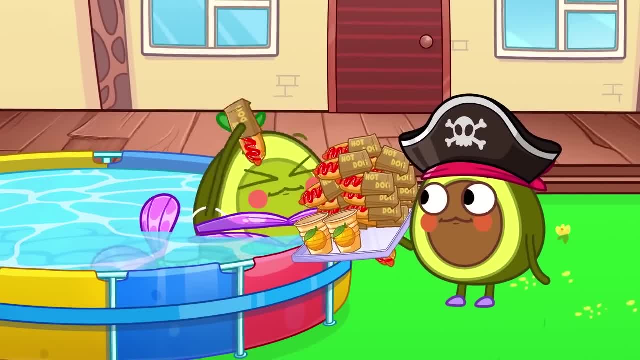 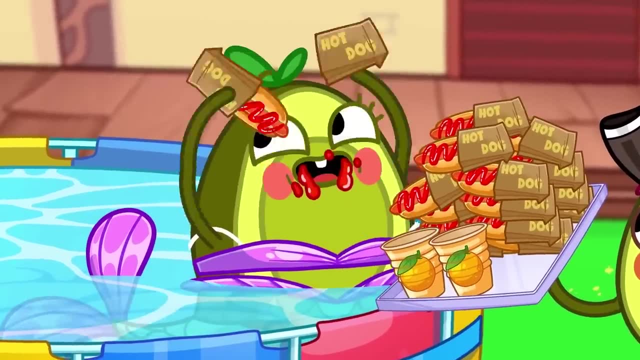 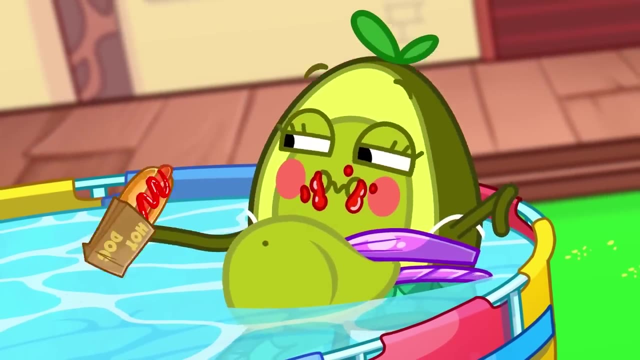 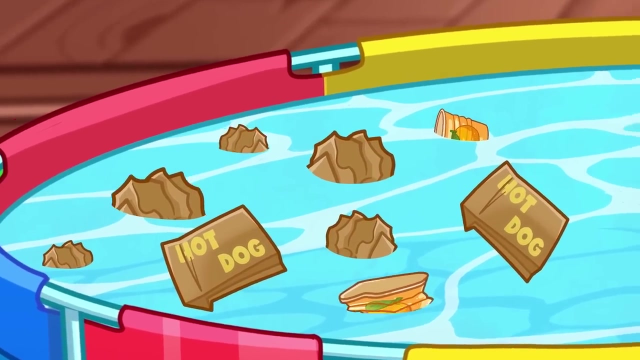 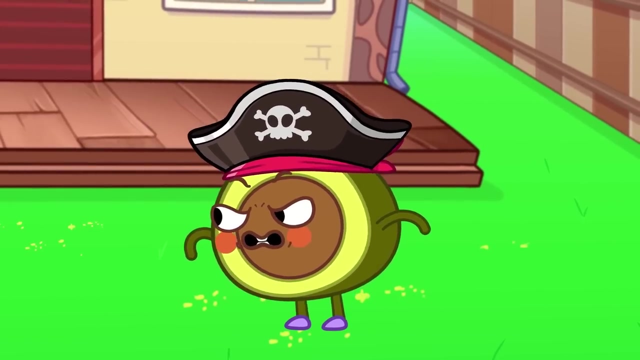 Okay, Penny loves hot dogs too. Oh no, She's eaten all of them. What a terrible mess. No, Penny, don't ever throw trash in the pool. What a terrible mess. Let's pretend that Pit's a pirate. 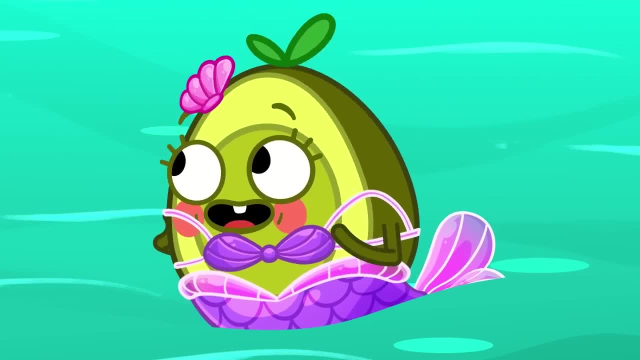 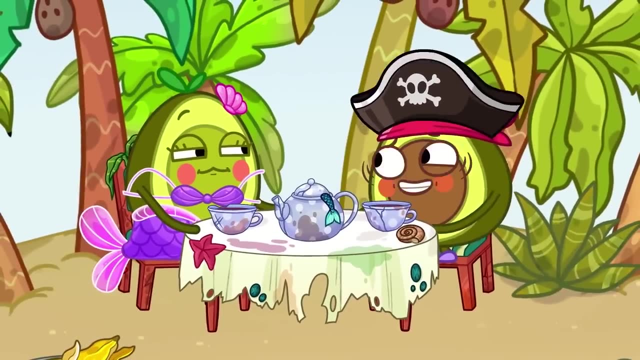 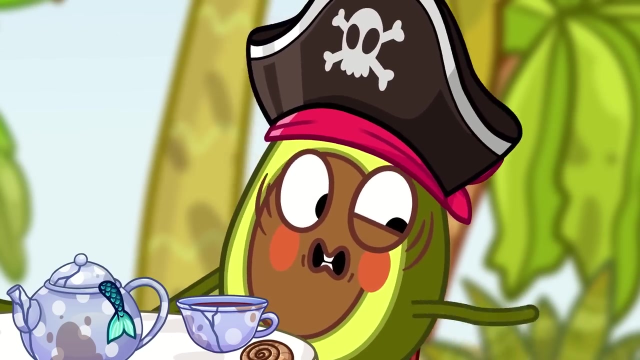 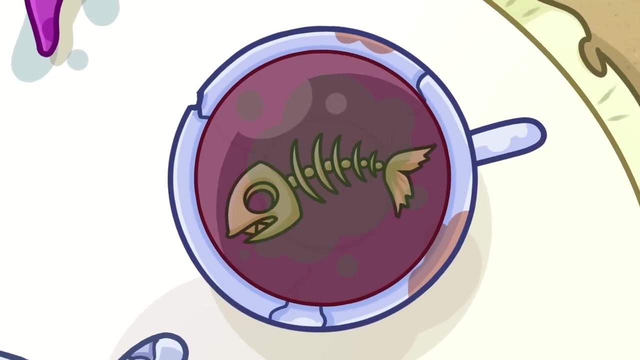 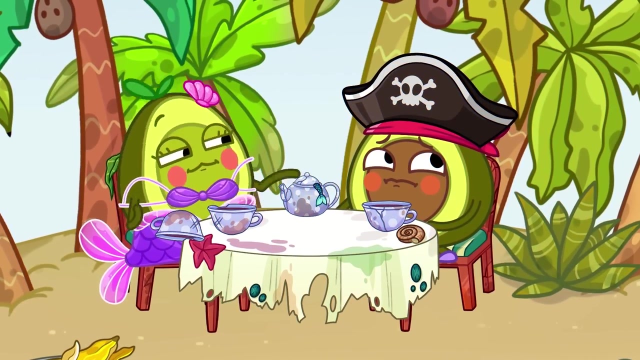 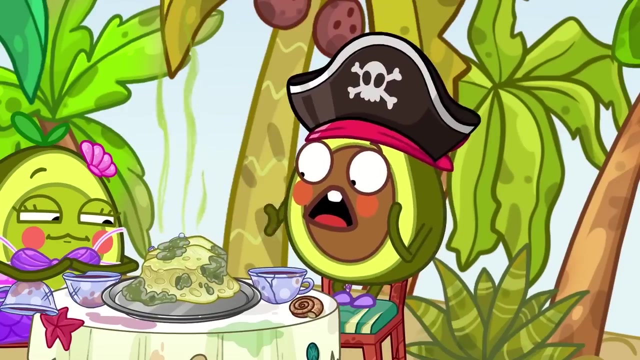 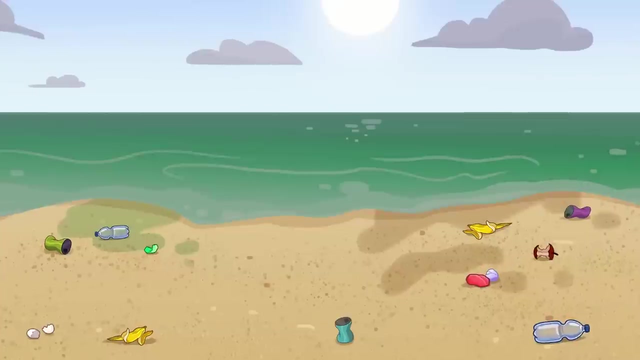 Do you want some ocean tea? Penny never cleans her island. It's really stinky. Eww Ow Ocean tea looks awful Yuck, But Penny loves it. Pit won't eat that, Pit. Pit, Come with me. 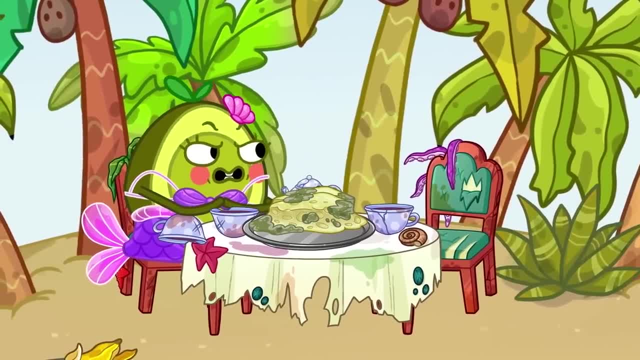 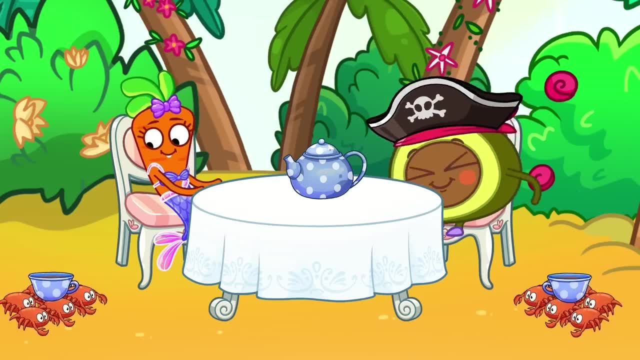 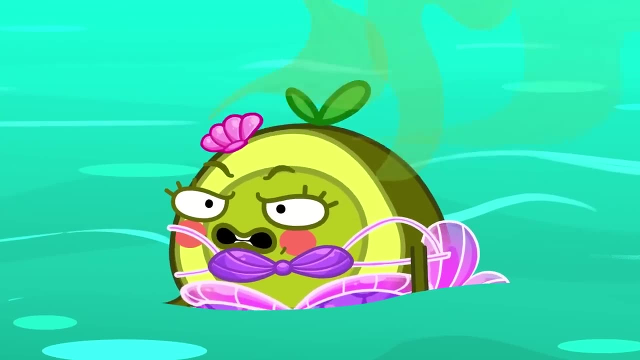 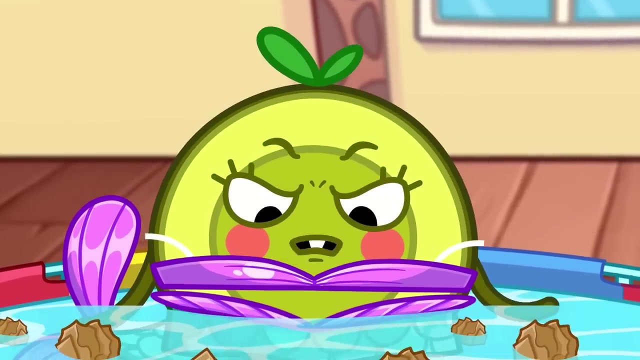 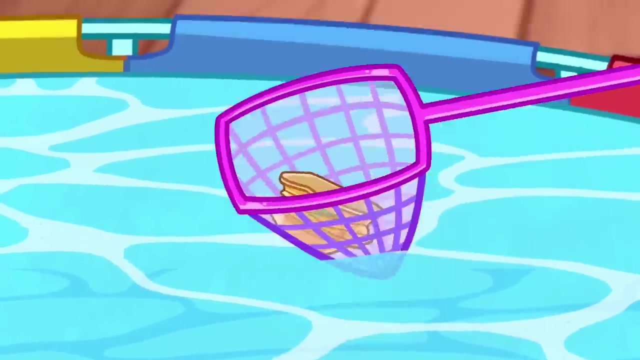 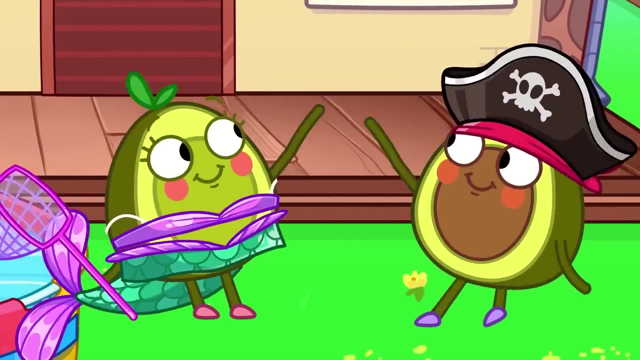 Yay, Carrot has a clean island. Try some tea Pit. Uh-oh, Penny isn't very happy. What are you thinking, Penny? Let's clean it. Yeah, Thanks for helping Carrot. You did it. 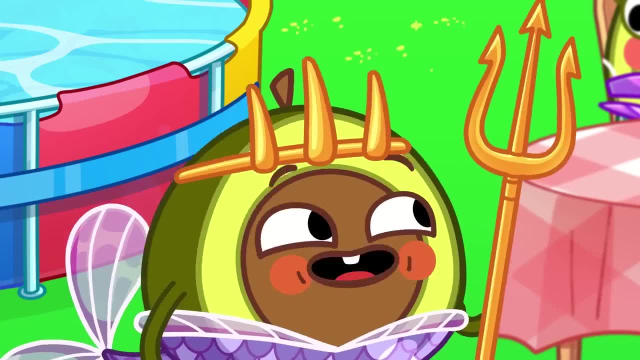 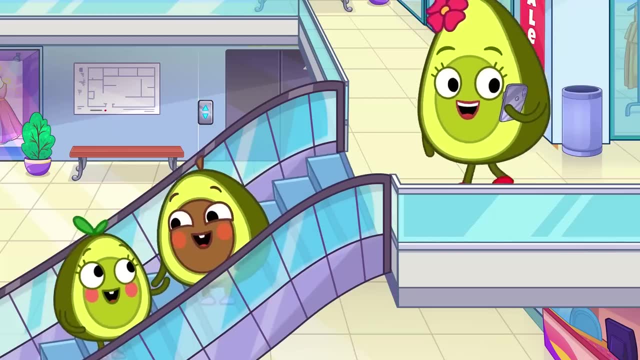 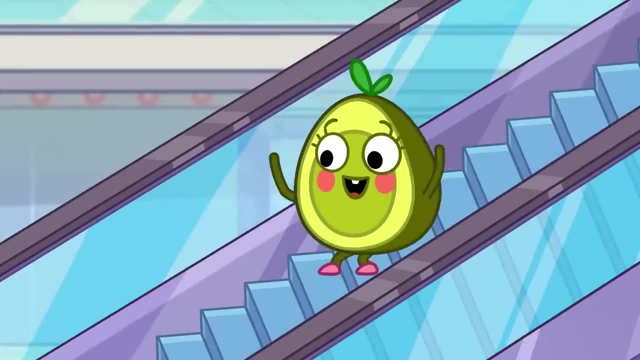 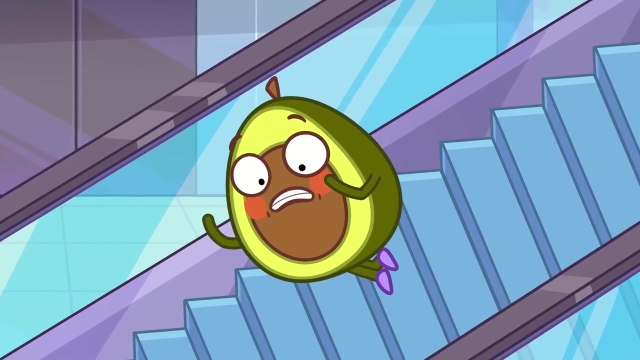 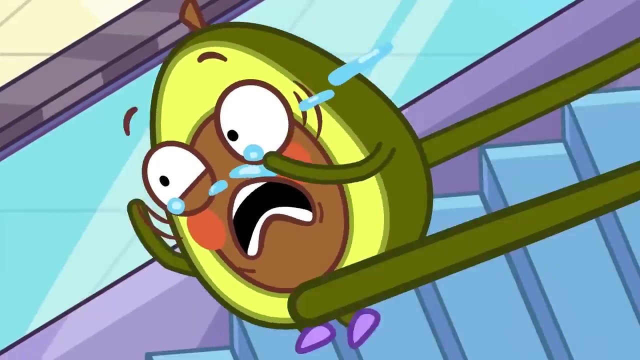 Now everything is nice and clean, Let's go swimming. What a great idea. Pit, Penny are at the mall with Mommy. Uh-oh, Careful, Playing on escalators is dangerous. Oh no, Pit is in trouble. Good thing Mommy was there. 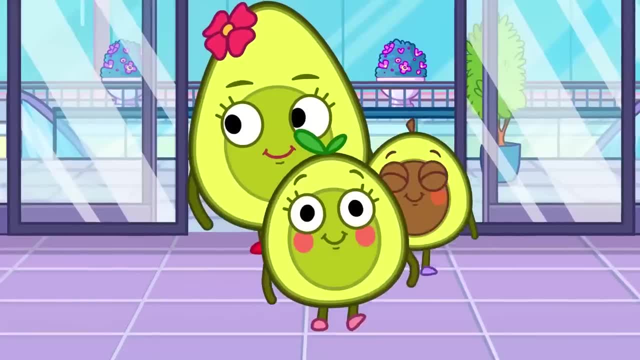 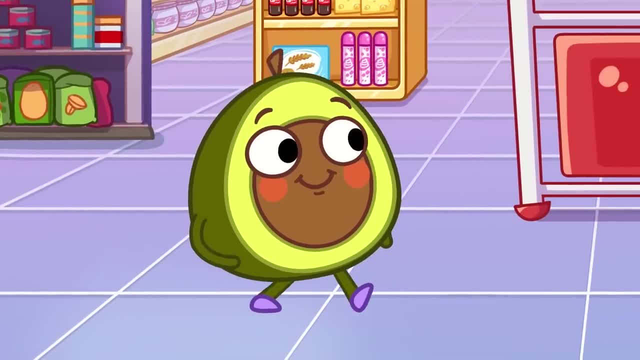 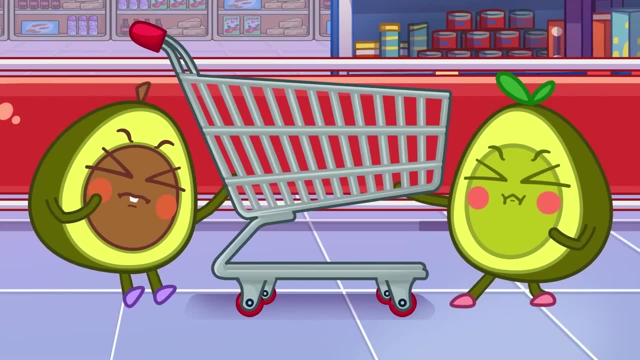 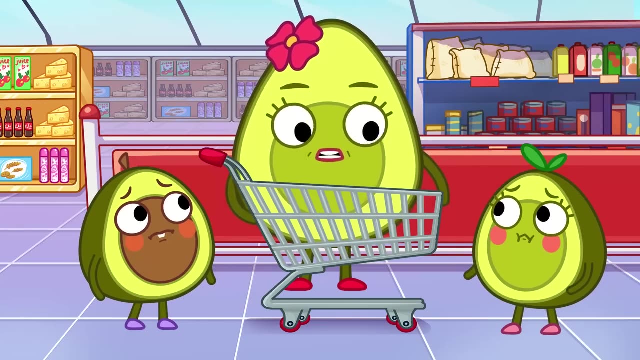 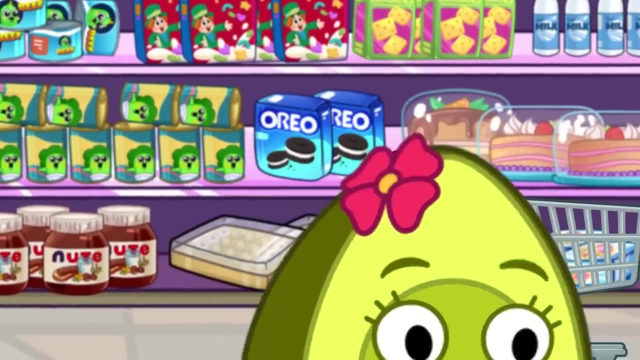 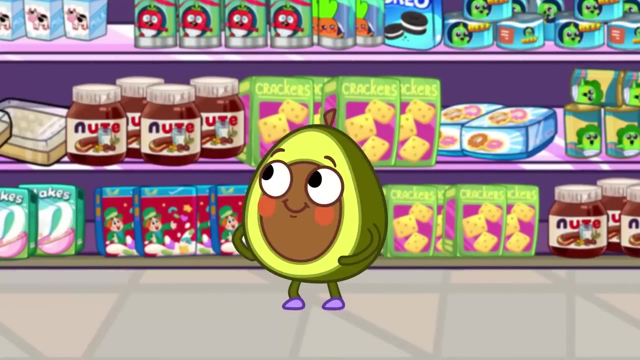 Where did Pit go? Here comes Mommy. You can't play with a shopping cart in a store. Mommy knows exactly what to buy. It's Penny's favorite cereal. It's Penny's favorite cereal. What are you thinking, Pit? 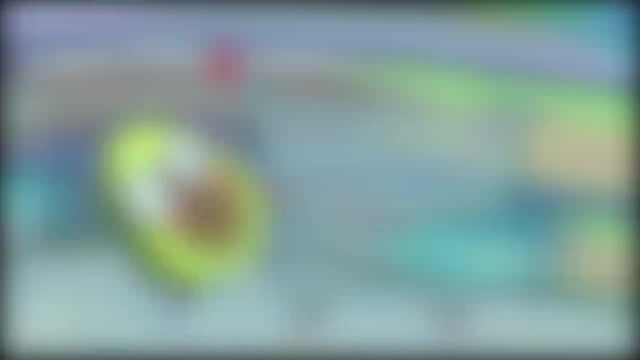 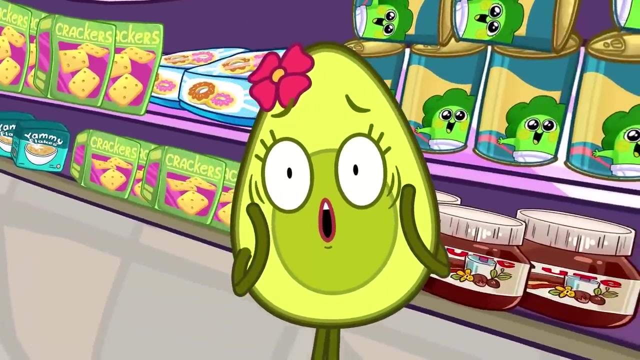 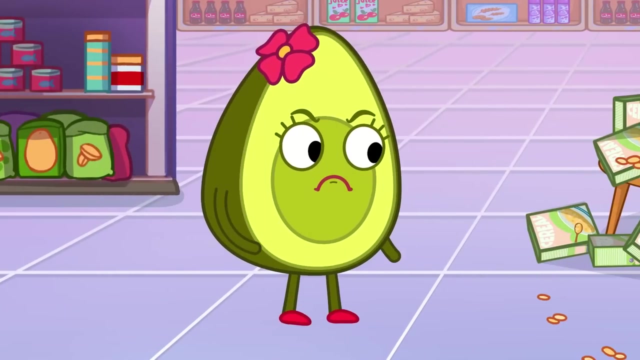 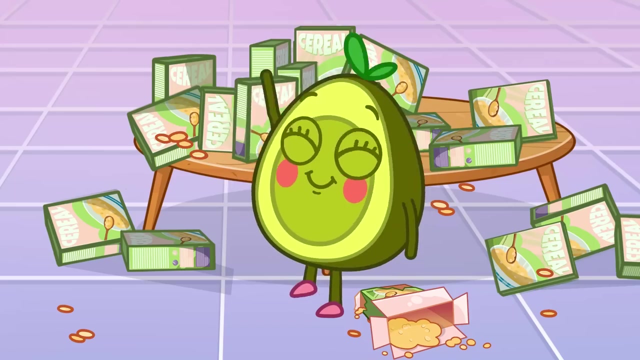 Pit, you need to be careful. Mommy has misplaced three things: The cart, Penny and Pit. Penny, Mommy is looking for you. You can't eat food in the store. Time to clean up your mess, Good job. 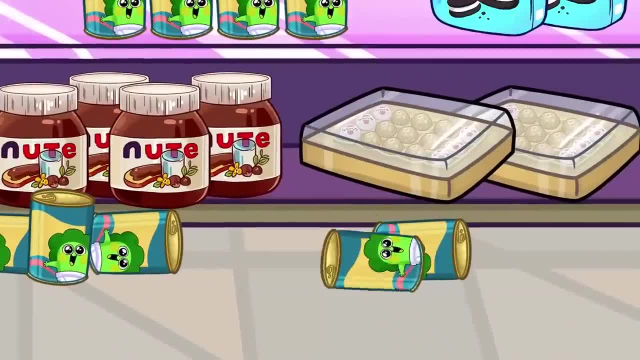 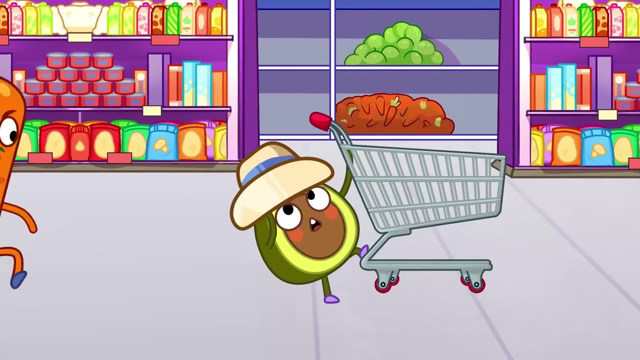 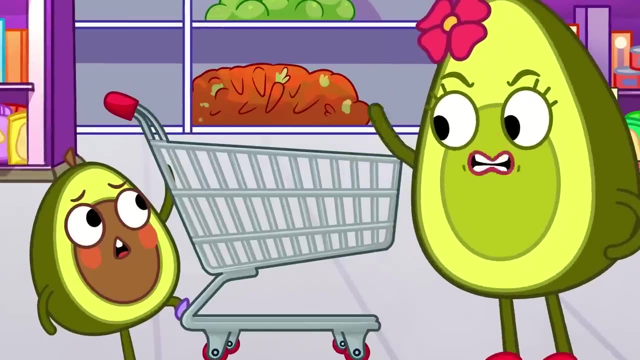 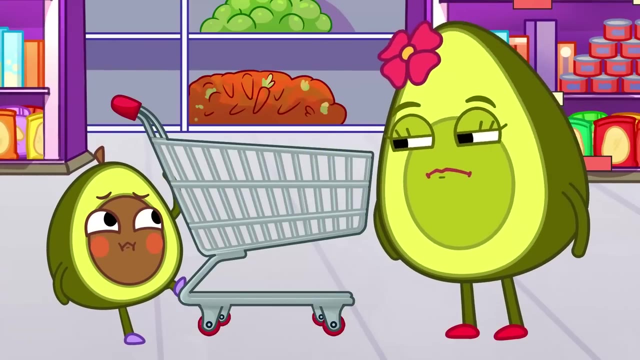 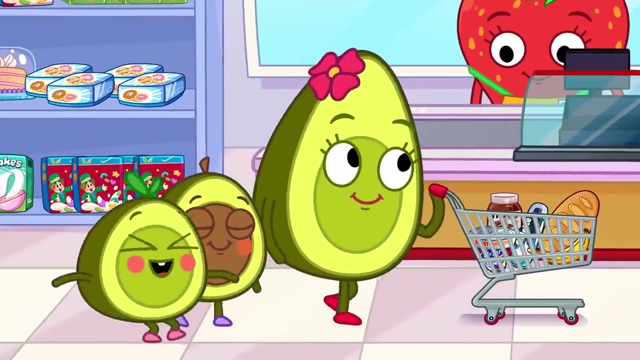 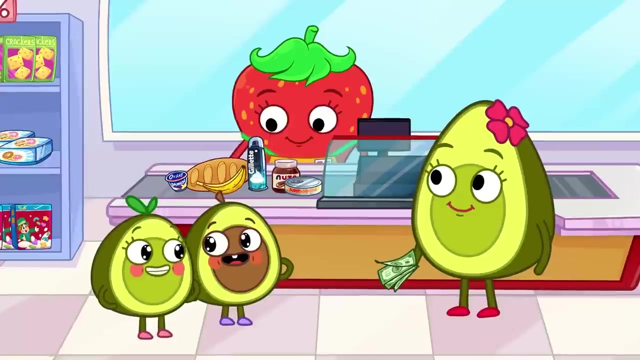 Good job, Pit. Mommy is looking for you. You can't run around with a cart in a store. Look at that mess. You better clean it up, Pit, Good job. There's one more thing to remember: You always have to pay for the products in the store. 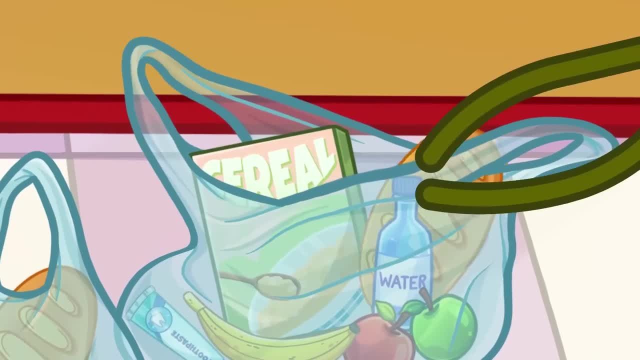 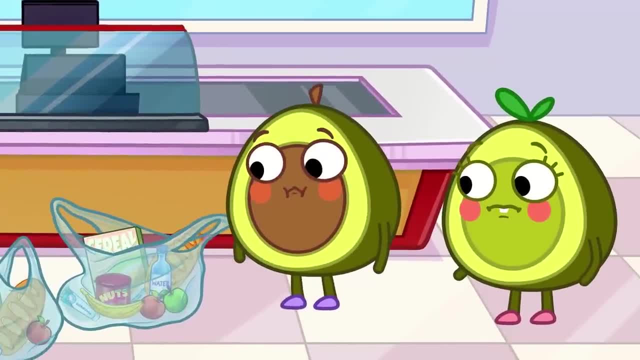 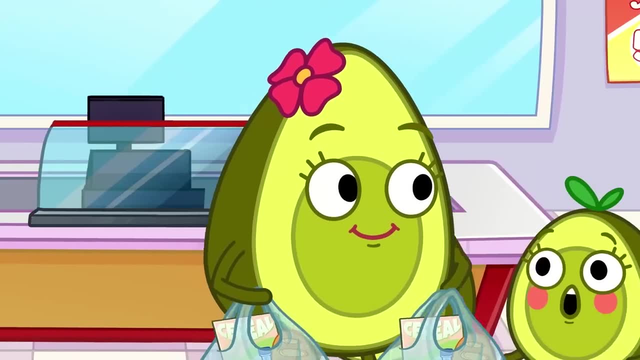 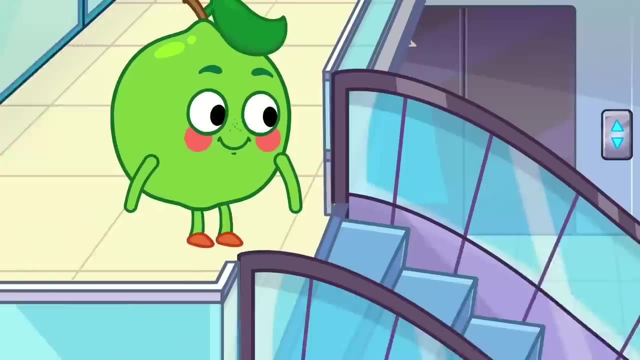 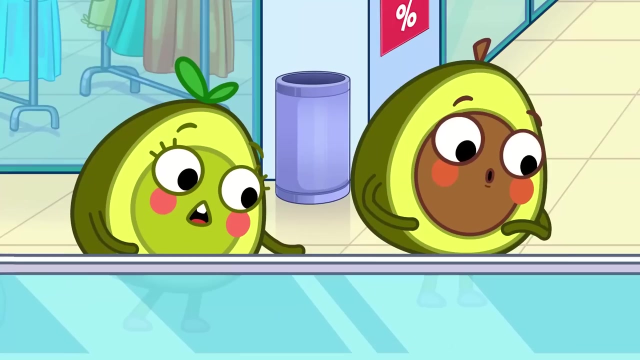 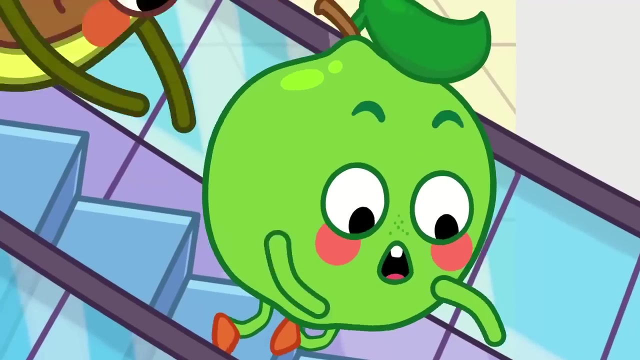 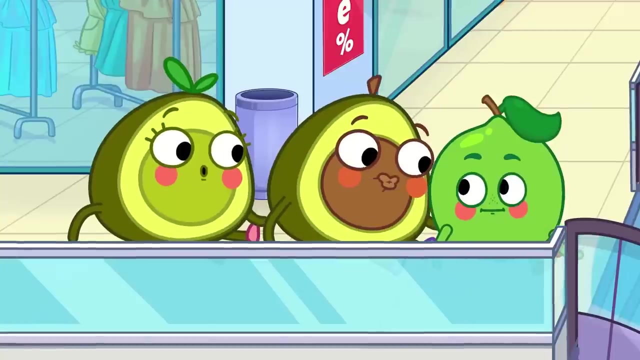 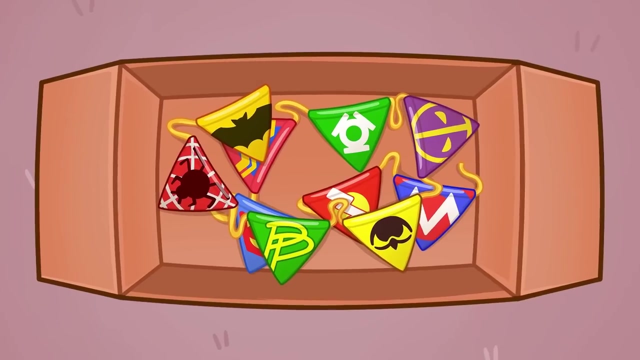 You always have to pay for the products in the store. Oh no, Lime is playing on the escalator. Lime, You're going to get hurt. You can't play on the escalator. Well done, Pit and Penny. Mommy is planning a surprise for Pit and Penny. 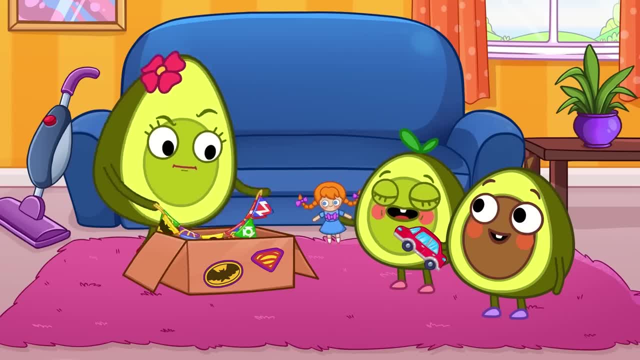 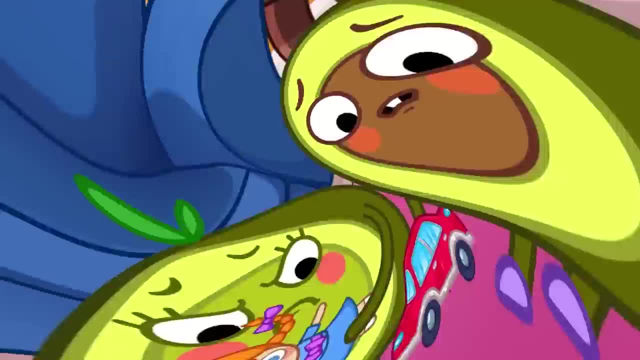 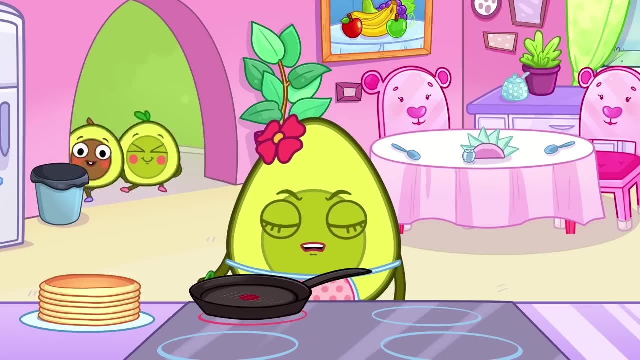 Shh. Mommy, Let's play Kids. I can play right now. I'm busy. Now, what will Pit and Penny do? Mommy is baking some surprise treats. Don't tell Pit and Penny. No, no, no. 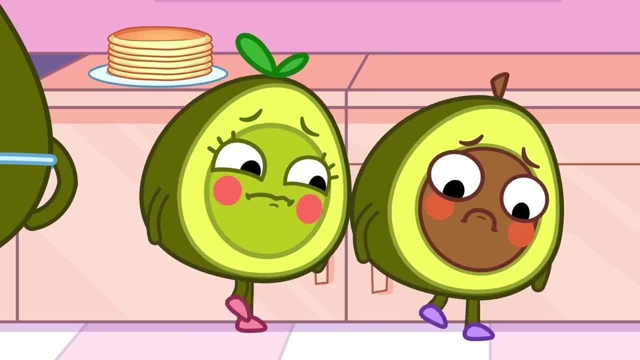 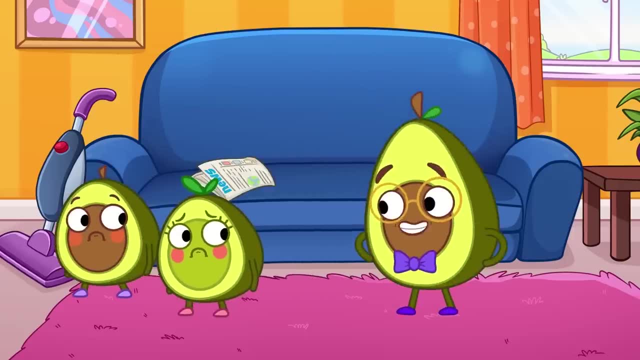 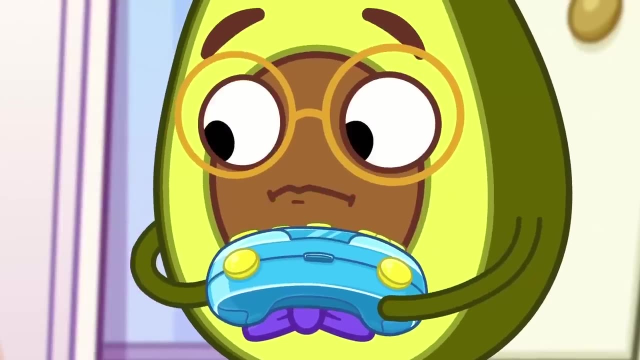 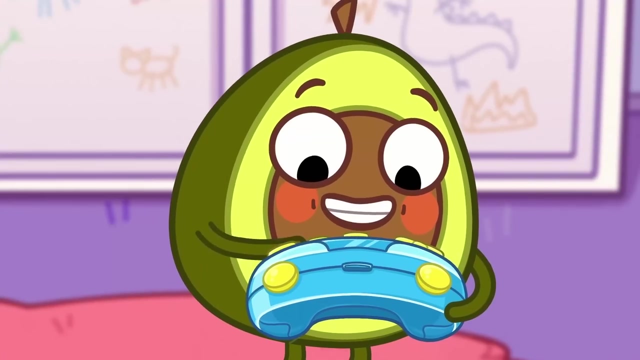 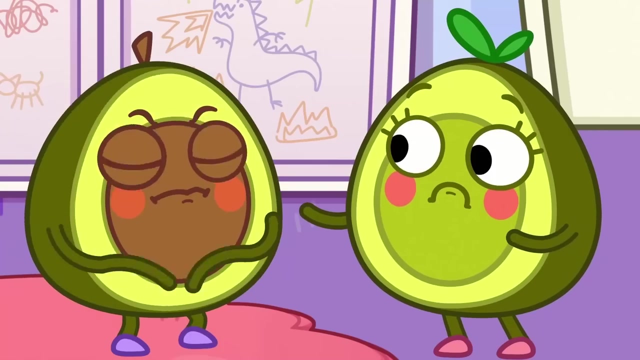 Mommy doesn't love us anymore. No, Maybe Daddy will play with you. Yeah, Kids, let's play together. Remote control cars are fun. Now it's your turn. Penny doesn't want to wait for her turn, And now the toy is broken. 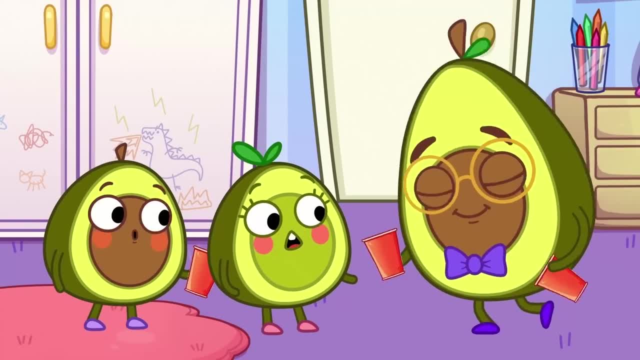 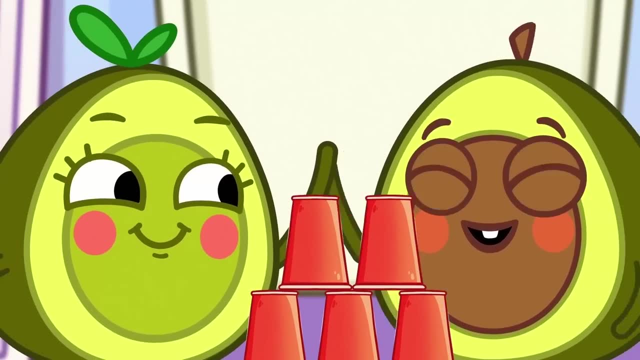 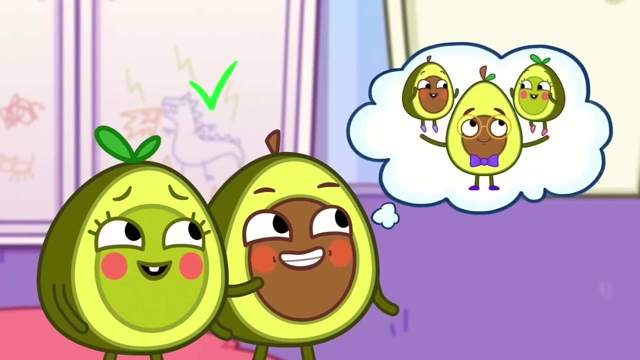 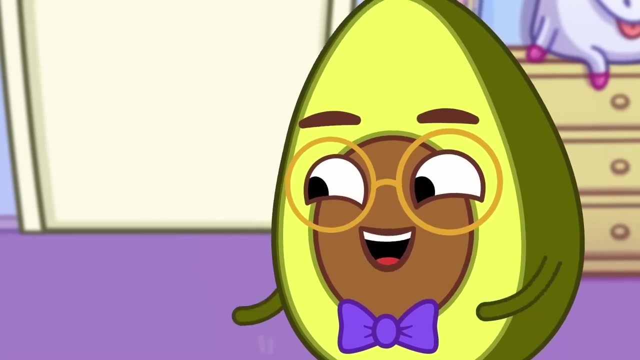 Daddy has another game they can play. All they need are some cups. It's a tower And Daddy has the final piece. Pit and Penny think Daddy is more fun than Mommy. Let's play hide and seek, Quick Run and hide while Daddy counts. 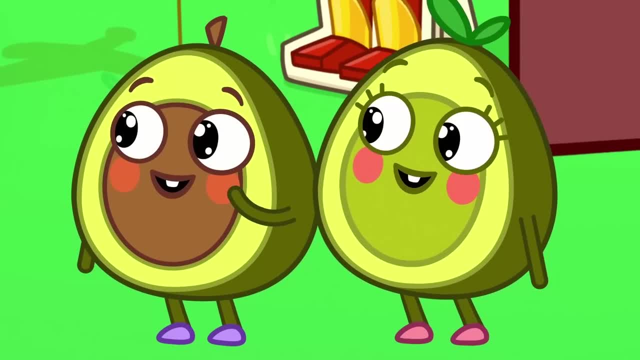 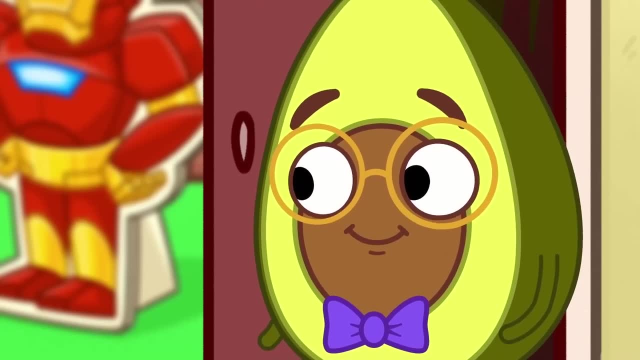 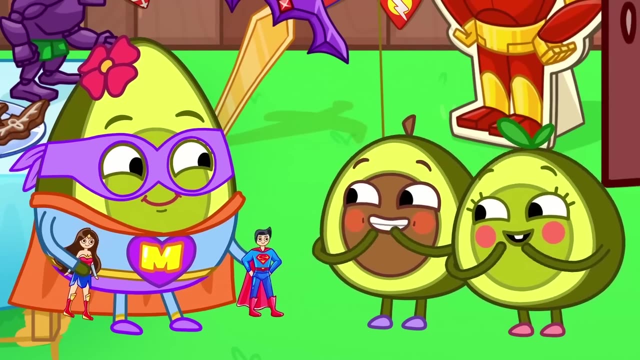 Huh, Look, Mommy is surprised, Huh, Surprise. That's why Mommy was so busy all day. Let's have some fun. Huh, Kids, do you have something to say? I love you, Mommy. 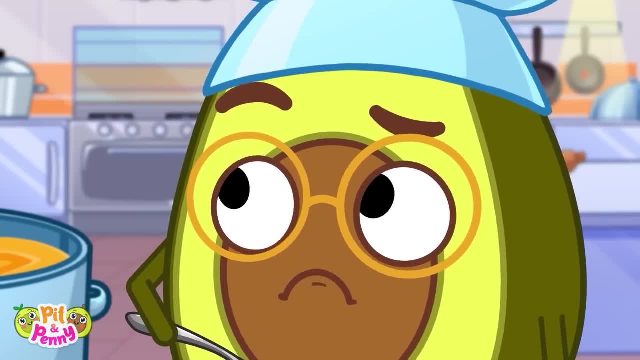 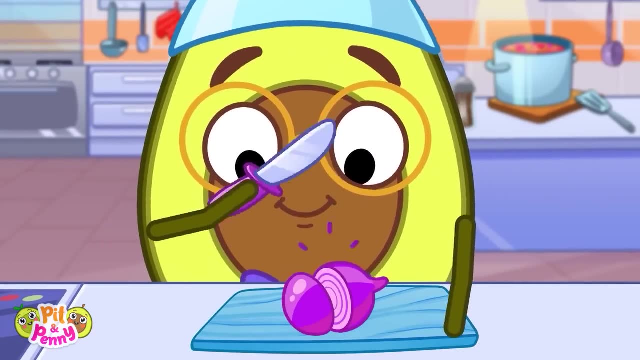 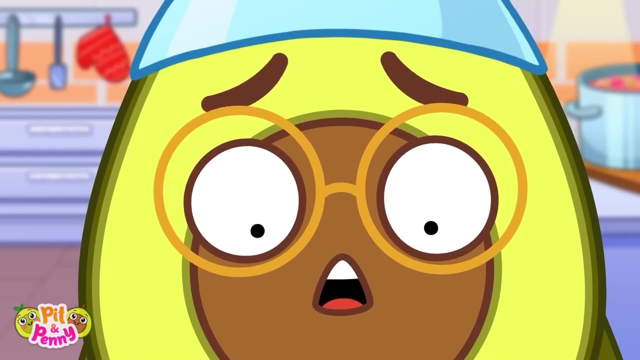 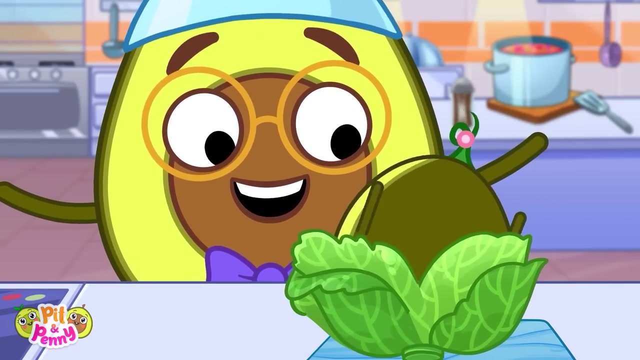 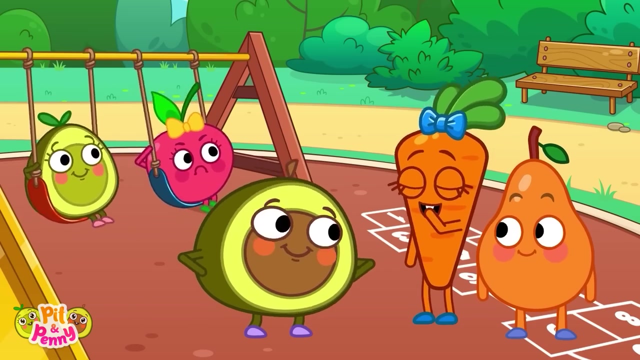 Daddy is busy cooking in the kitchen. What will make the sound better, make the soup taste better? Carrots, Onion. Why is the cabbage moving? There's a cute little baby inside. That's how we were born. What do you think, Carrots? You were wrong. 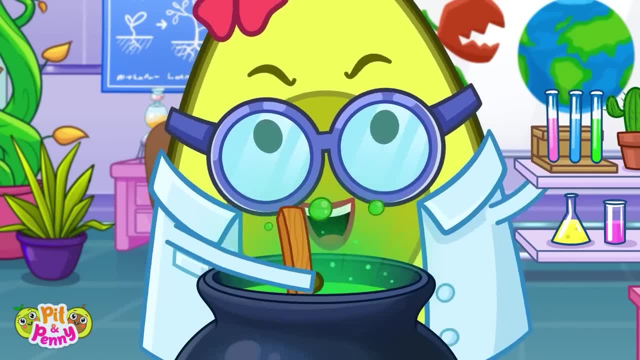 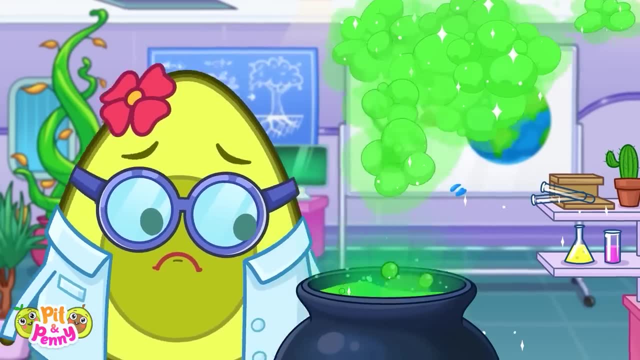 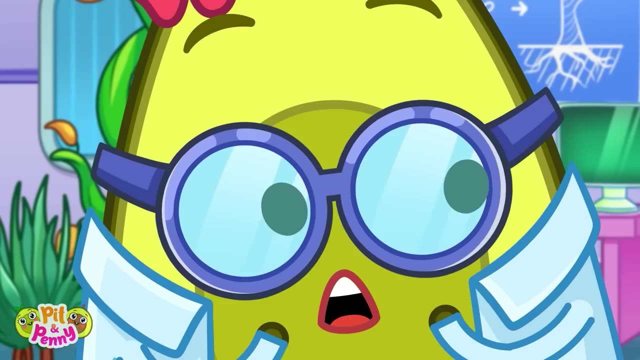 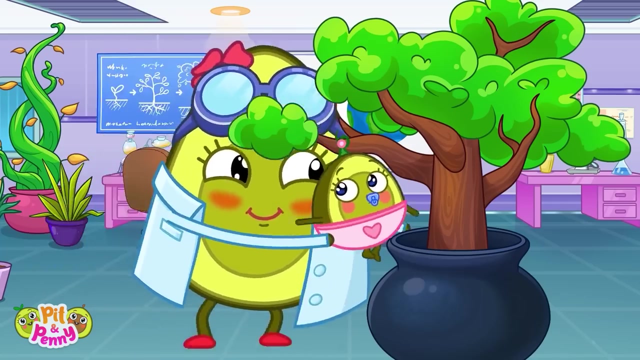 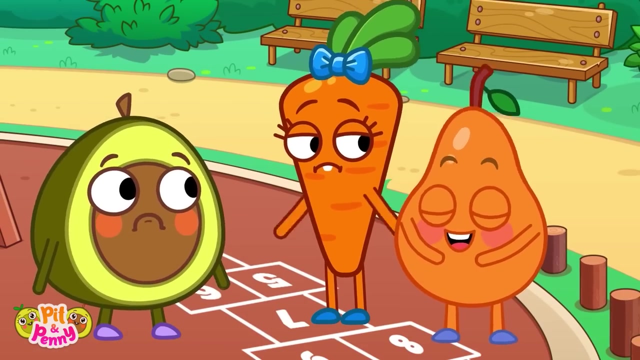 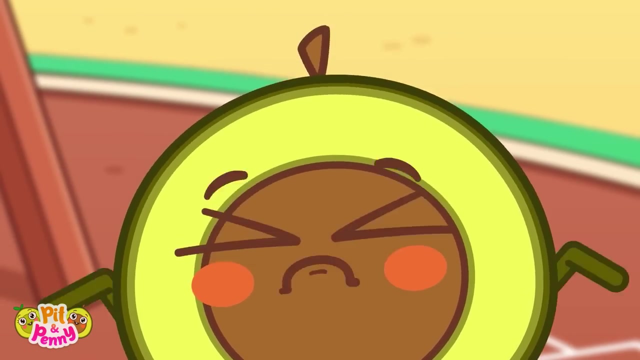 Listen. Mommy's in the lab making a potion. Oops, There's a baby in the tree. Oh, That's how we were born. Oh Pit, Oh Carrot, That's not where babies come from. What are you doing? We are wondering about how we were born. Does Pear know Listen? 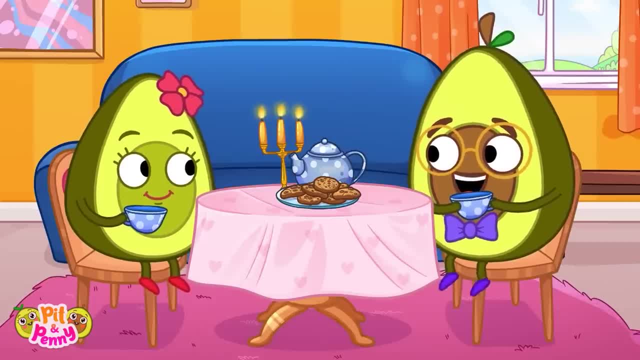 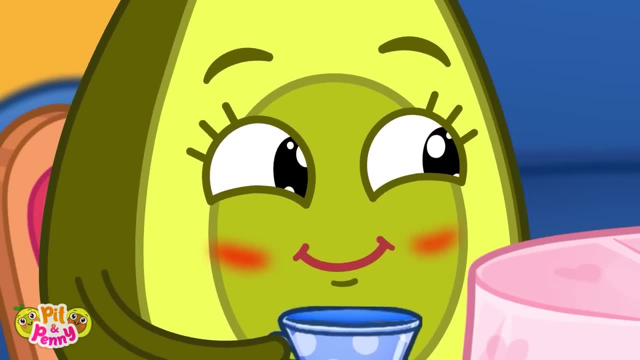 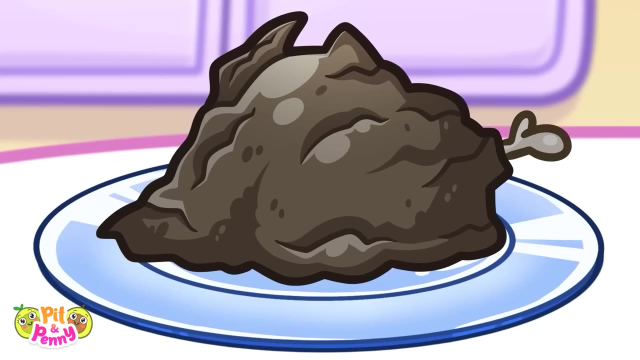 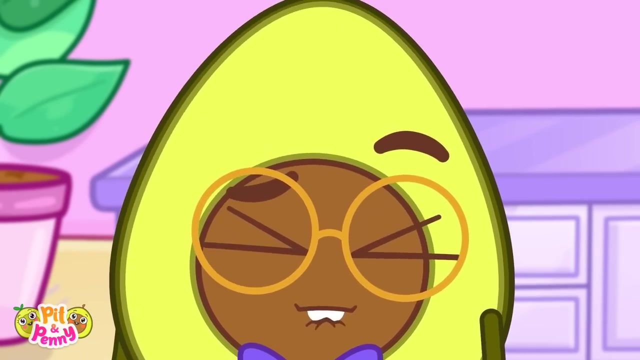 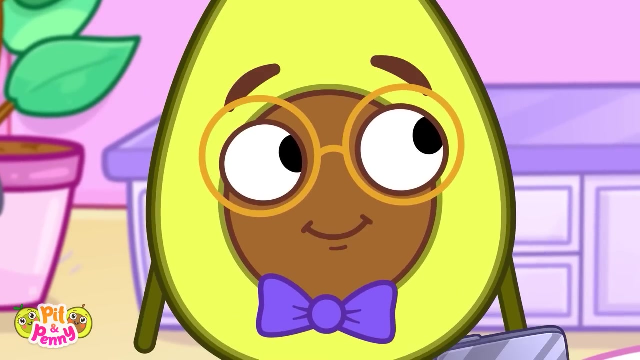 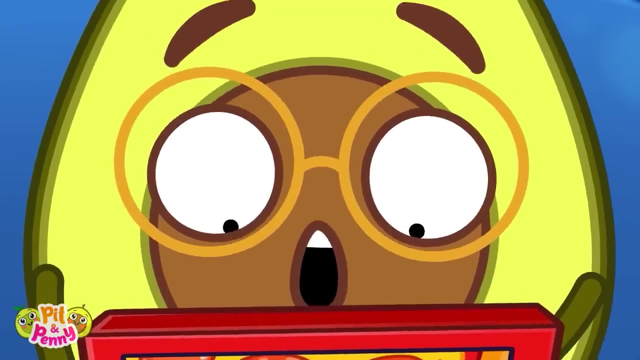 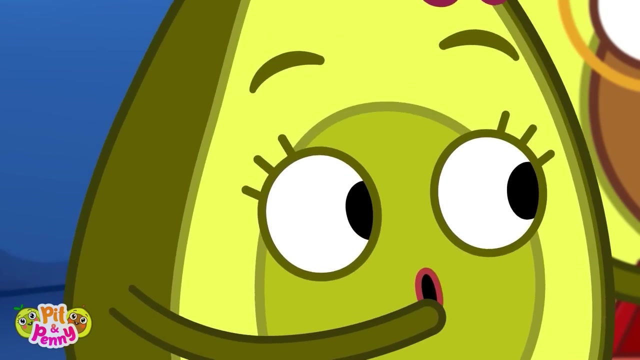 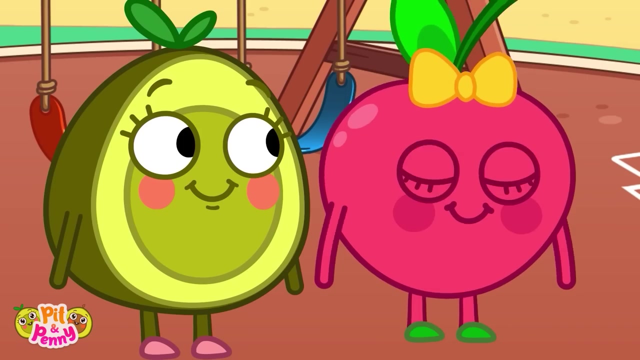 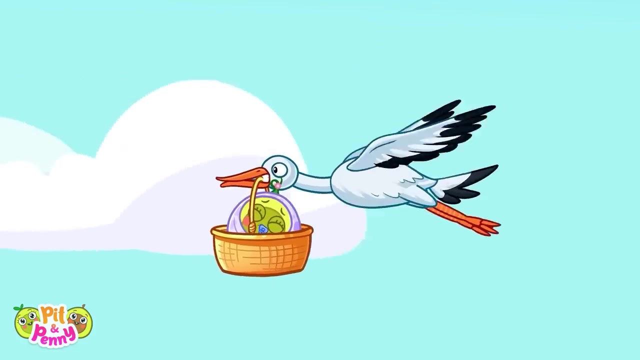 to me: Mommy and Daddy are having a nice dinner. Daddy, your food is burning. How was dinner? Now, what will you eat? Mmm pizza? Oh, It's a special delivery, But that's not where babies come from. That stork is carrying a baby. 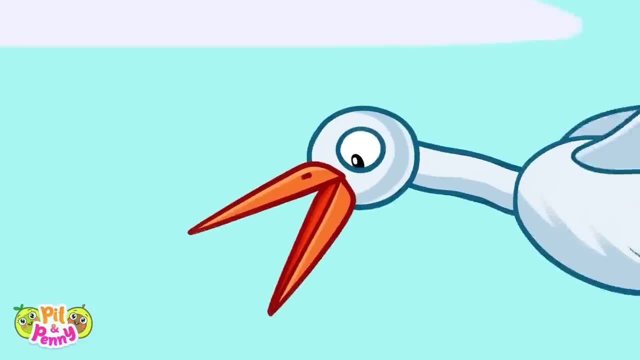 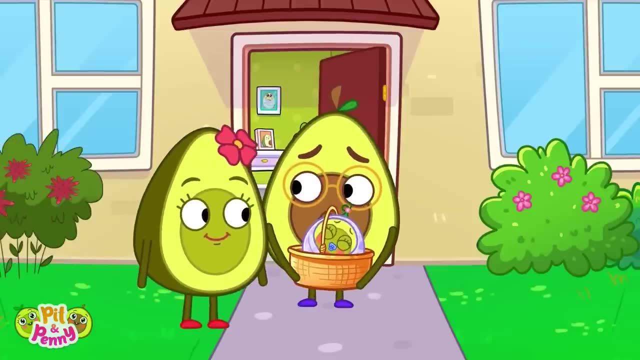 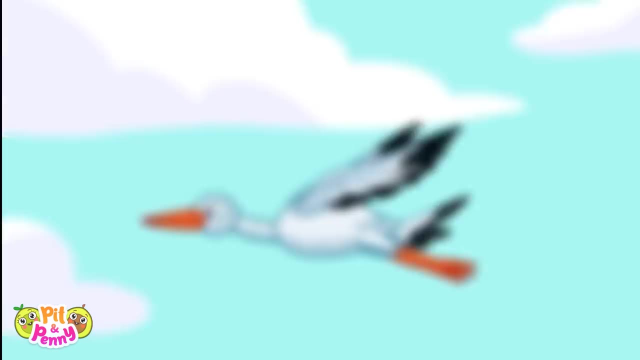 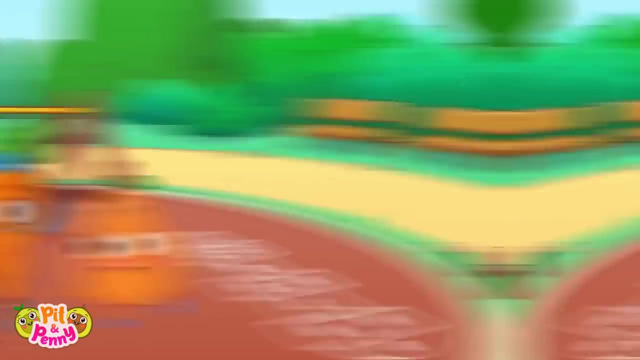 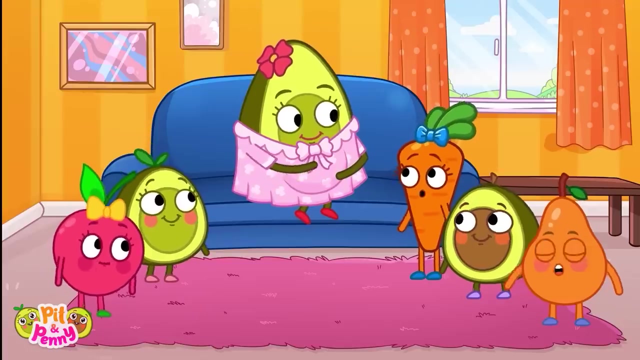 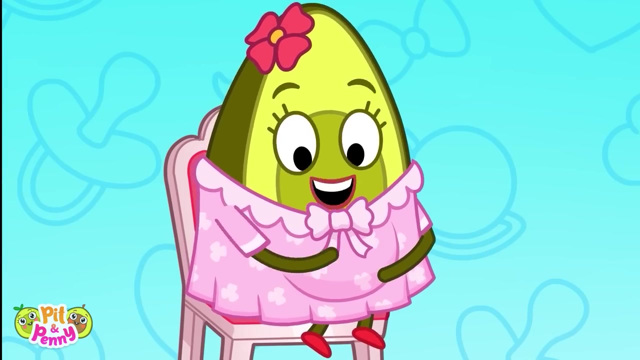 in a basket. Watch out, Good catch, Daddy. Maybe Penny knows. Follow me. The truth is that we were born from Mom's valley. That's right, Penny, Really Yes, My valley was a home for a little baby for a few months. You were there once too. 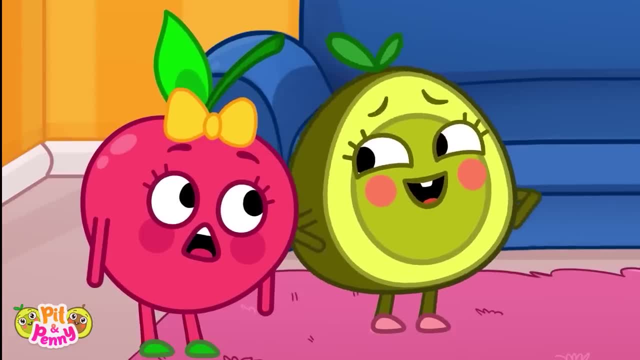 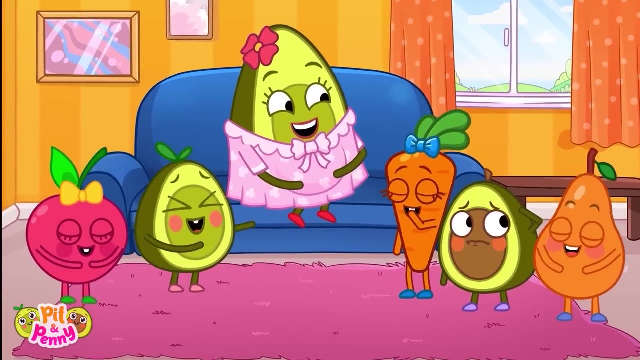 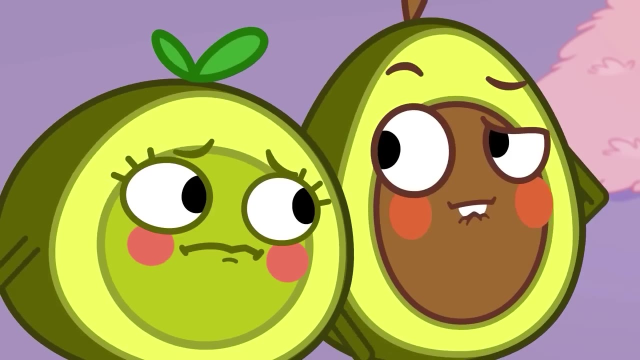 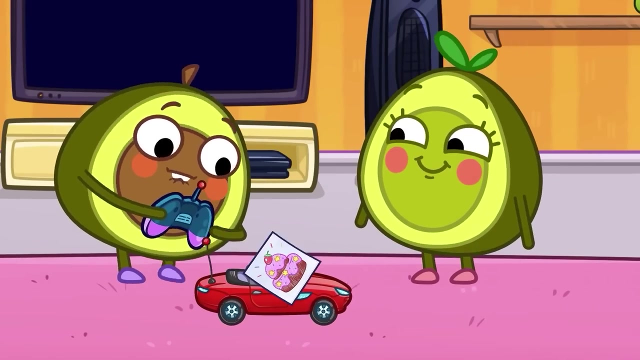 That's right. We all started life in a mommy's valley. I thought you had a big valley because you ate a lot. Oh, Pit Baby is sleeping. Hi, Hi, Hi Hi. Pit and Penny have a special note for Mommy. 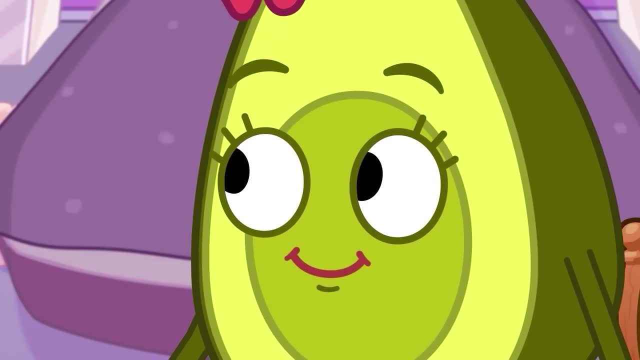 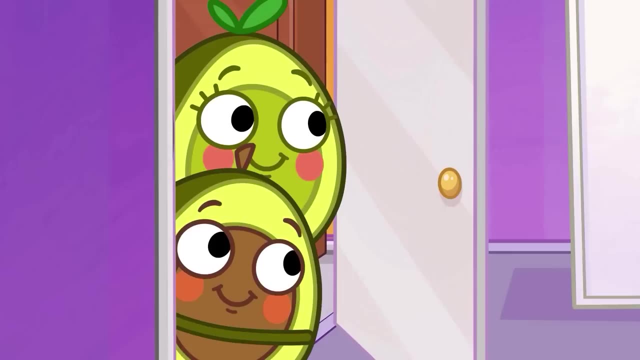 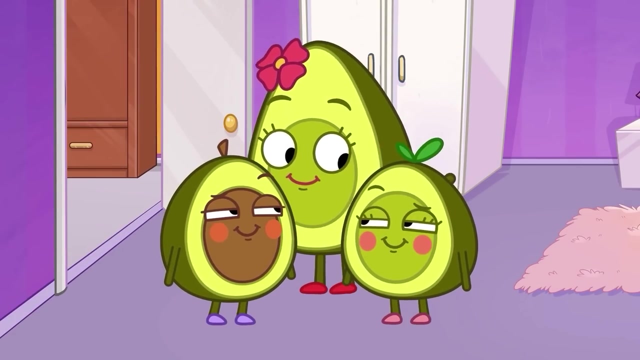 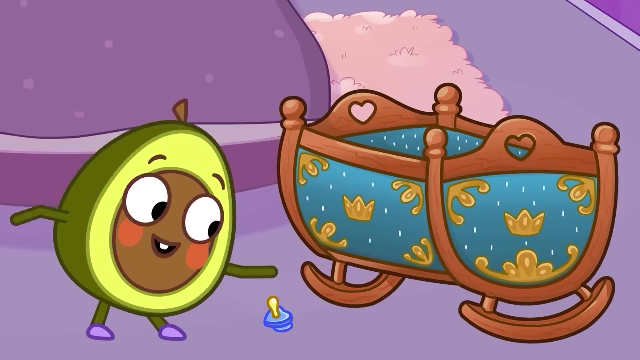 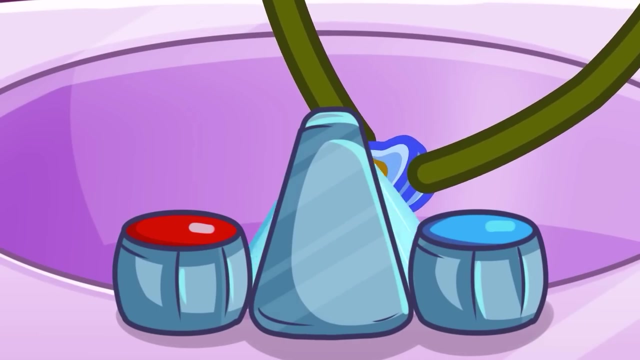 What do they want? Do you want some cake? Then you'll have to babysit your little sister, But it's a lot of work. Yeah, Yeah, Why is Baby crying? She lost her soother. The soother was dirty and needs to be cleaned. 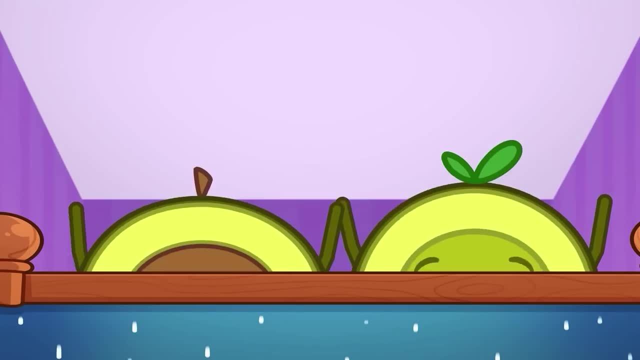 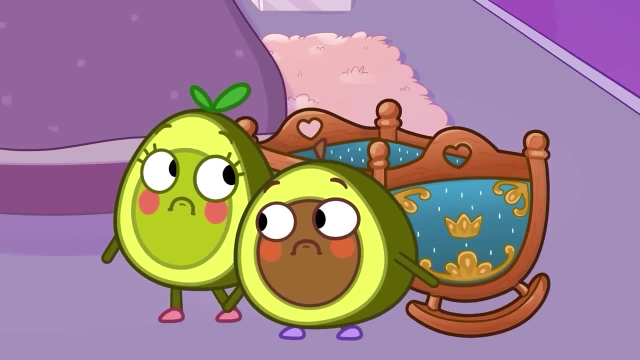 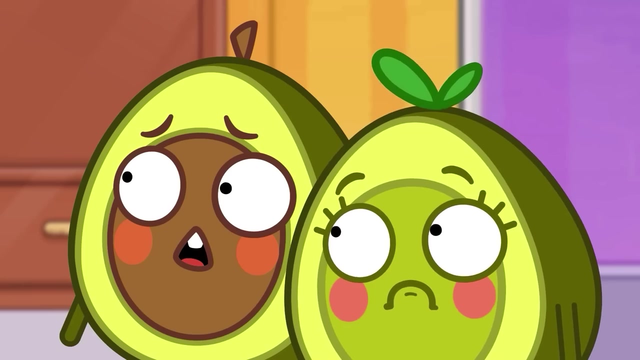 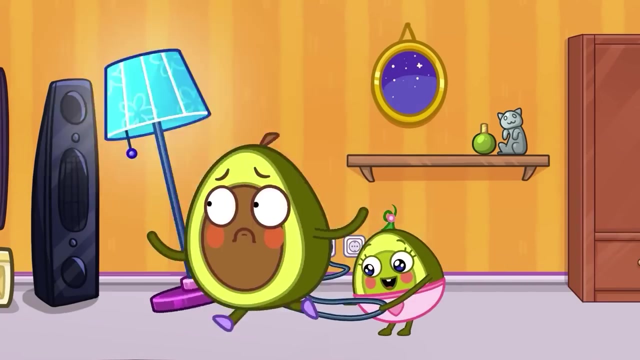 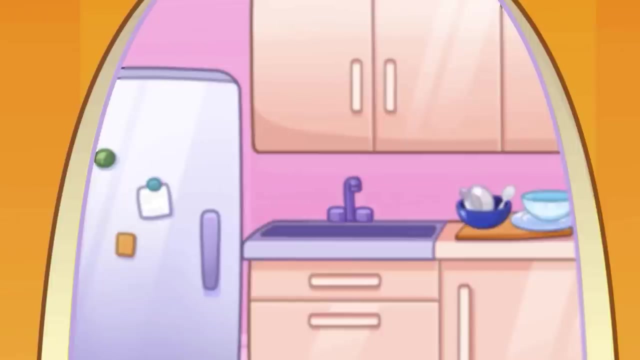 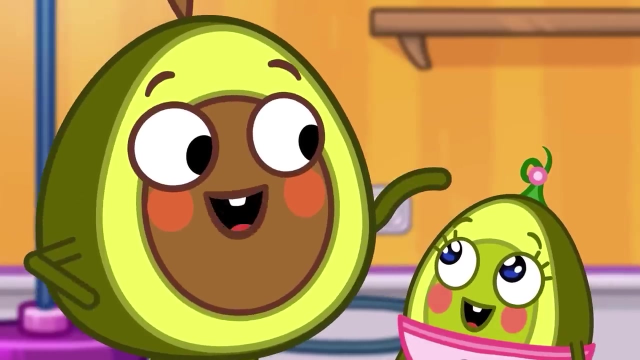 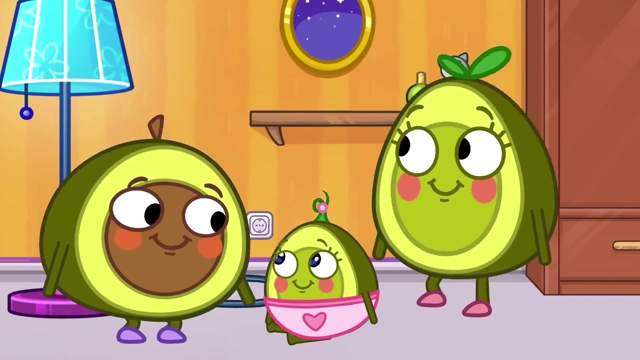 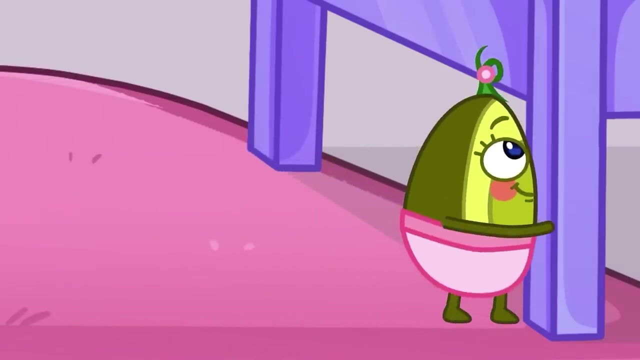 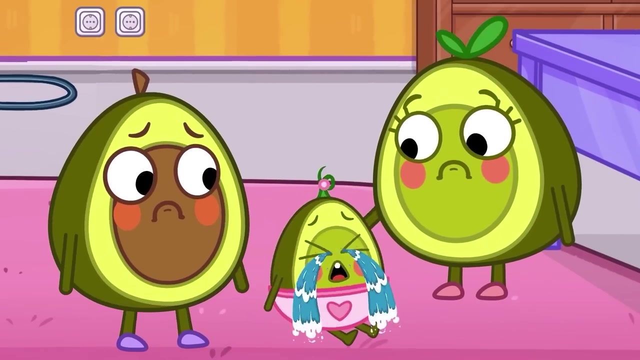 Good job. Oh no, Where did Baby go? Hurry, She's playing with the cord. Outlets are very dangerous, That's right. You can get hurt. Now what's Baby up to? Oh no, The scissors. Scissors can hurt you. 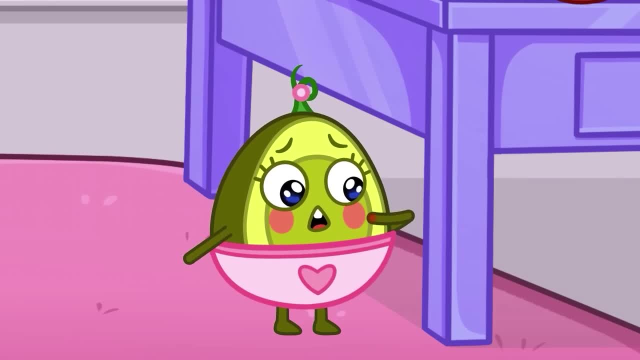 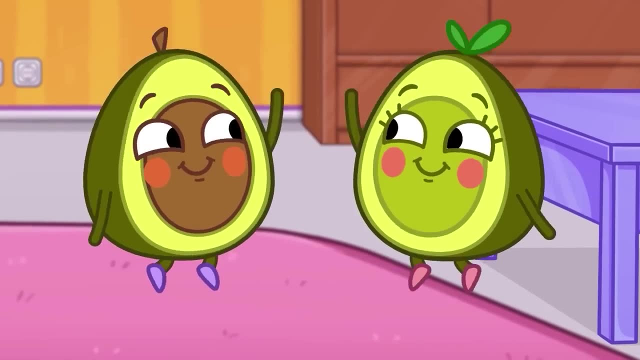 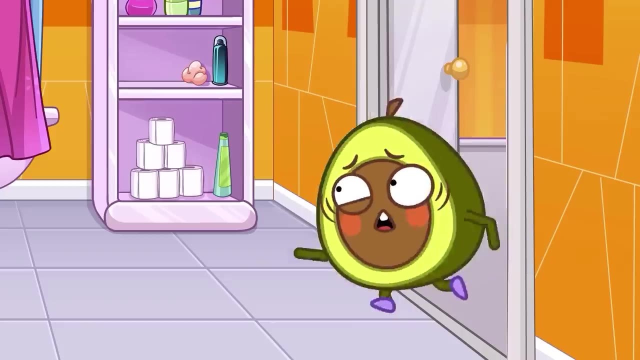 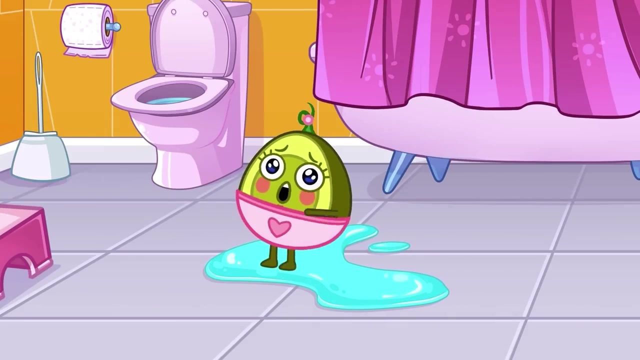 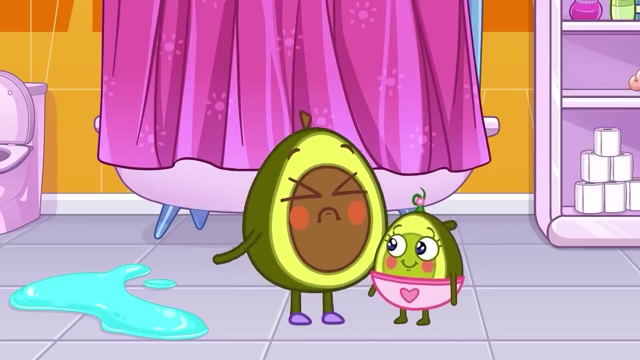 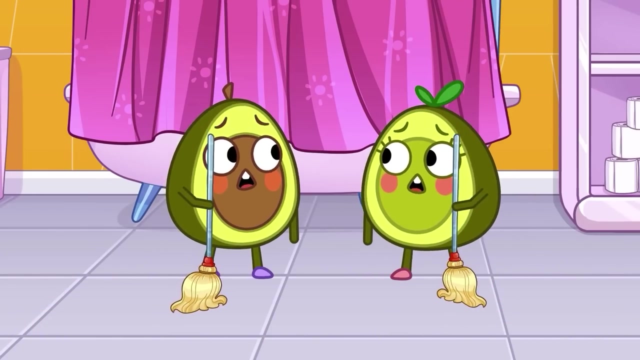 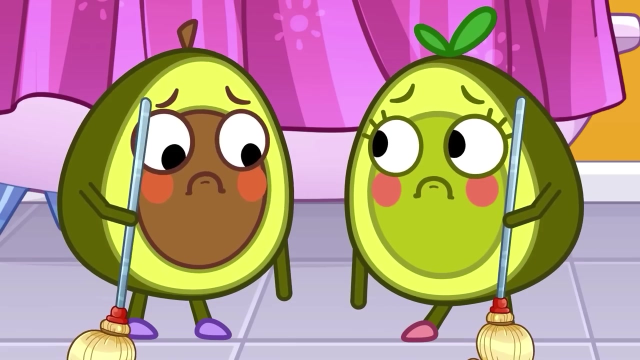 That's right. Scissors are sharp. Now Baby's in the bathroom. Quick, She's going to slip. Phew, You can't walk on wet floors. Now it's clean and safe. Being a mom is so hard. Now where did Baby go? 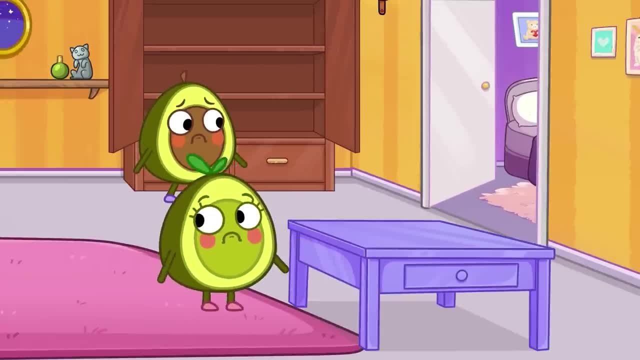 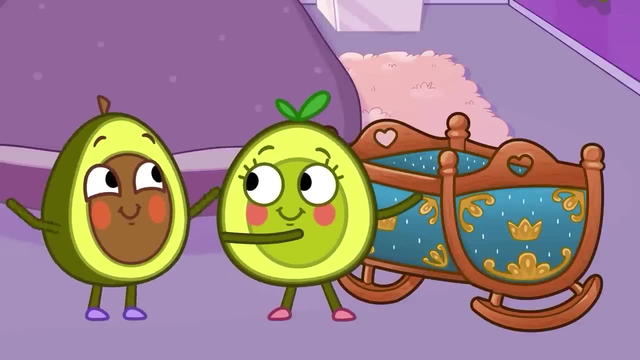 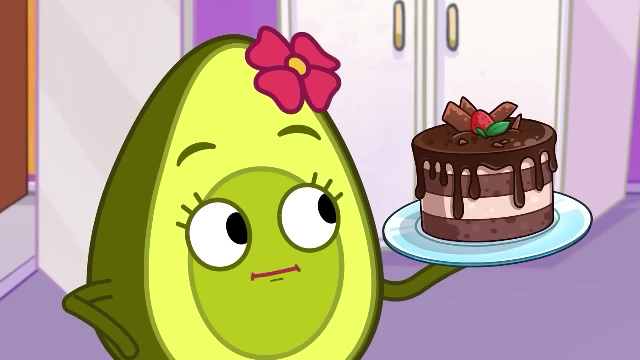 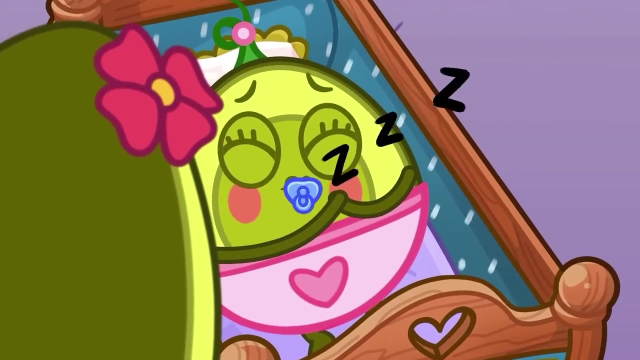 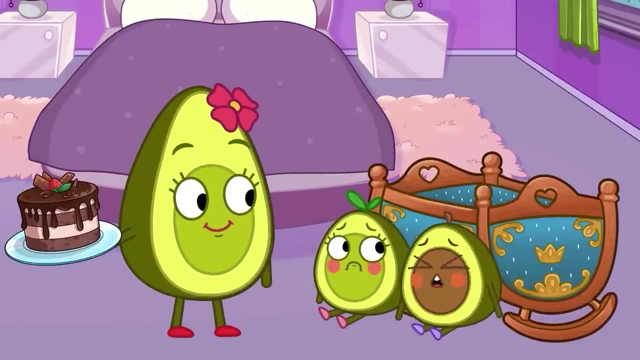 Not in the cupboard, Not under the table. She's asleep in her crib, Ben, She's here. Oh Pass, Look what Mommy has, And here is your cake. Oh, you're my superheroes. We won't be superheroes anymore, Mommy. 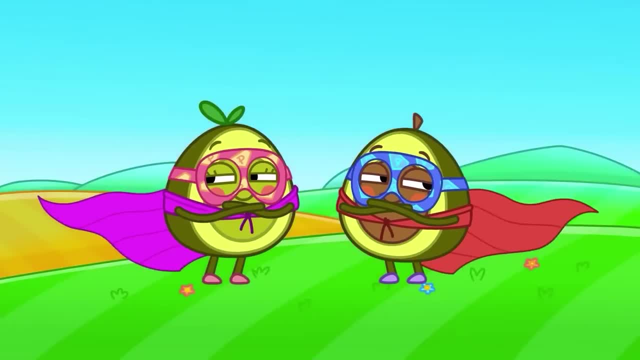 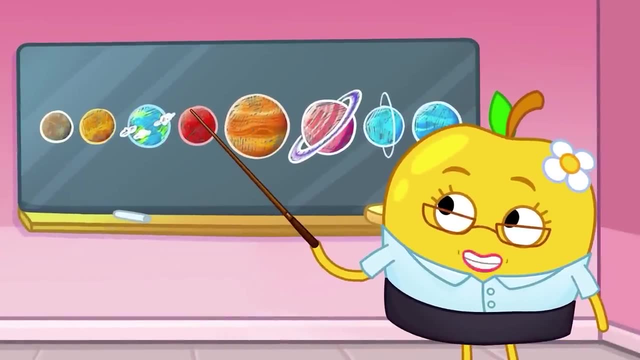 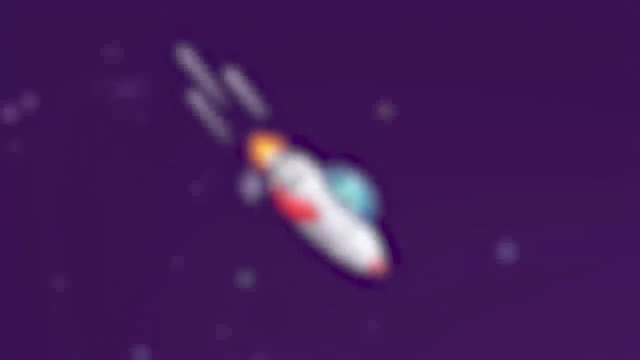 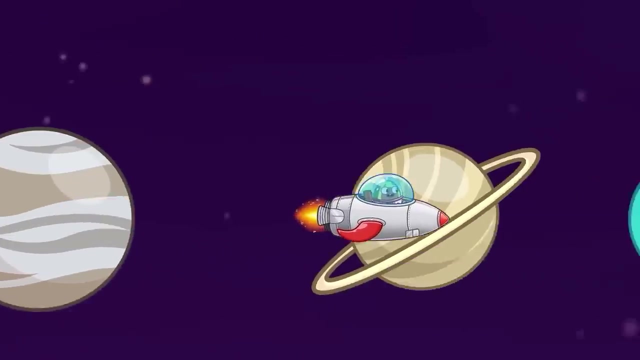 Are you sure? Maybe just one more time, Miss Apple. what will we be learning Today? we'll study the planets, But someone is snoring. It's Pit. He's dreaming, he's an astronaut And he's exploring the planets. 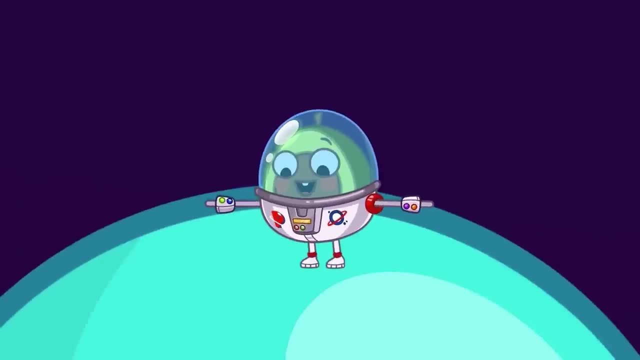 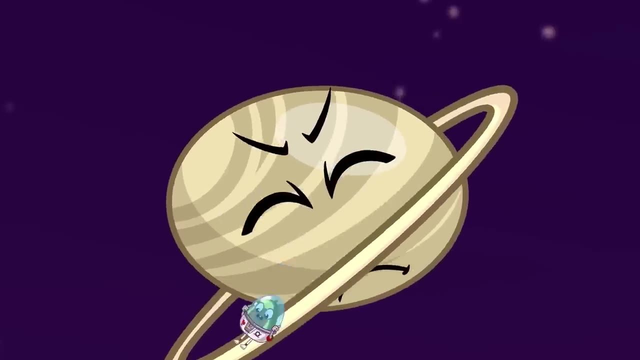 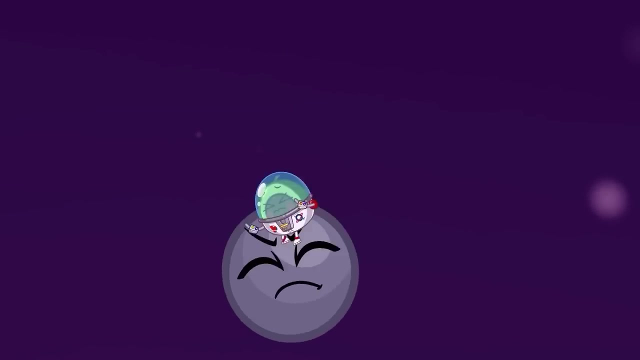 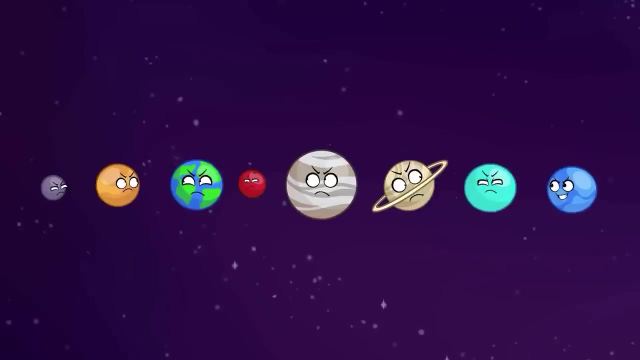 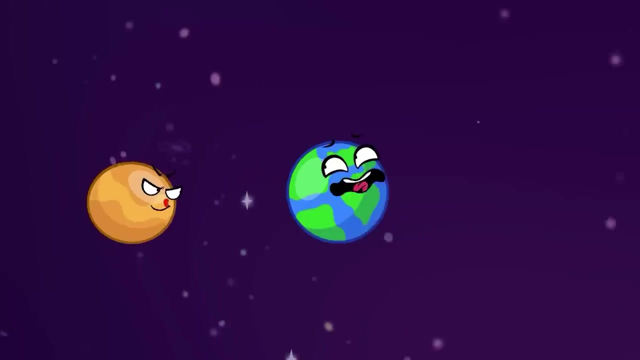 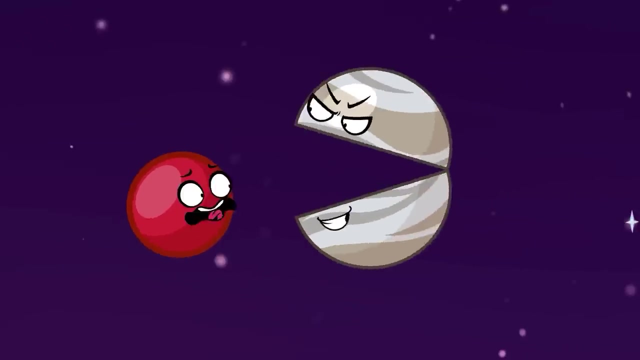 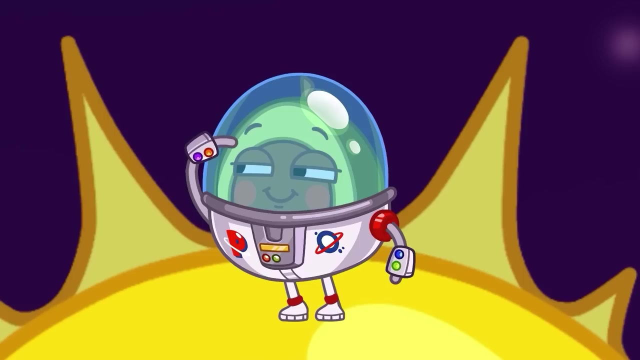 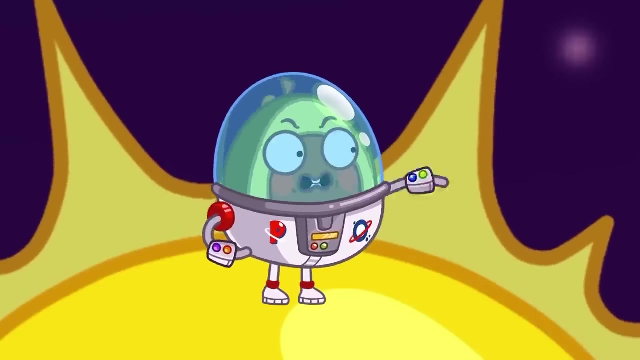 Tata, Oh, Yee-haw. But the planets, Oh, They don't seem happy, Poor Pit. Why are they so unhappy? Oh no, The planets are hungry. Help Pit, There's only one planet left. Hey, Get them back. 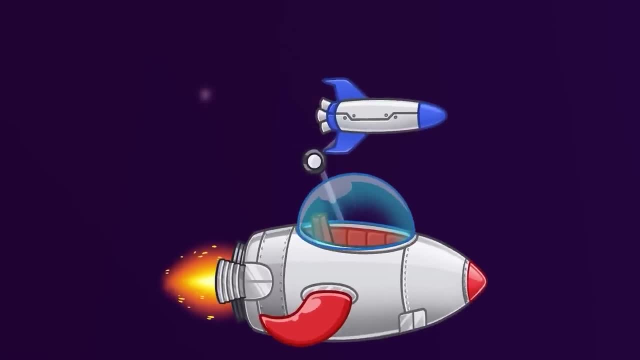 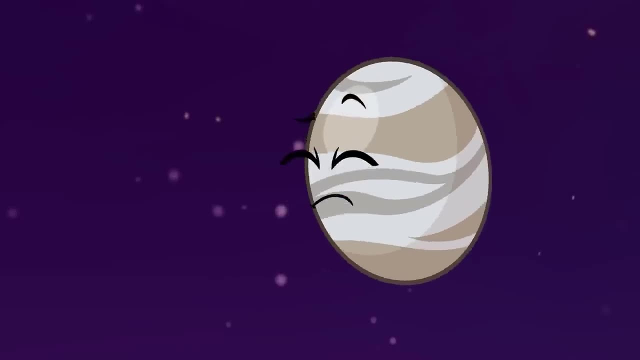 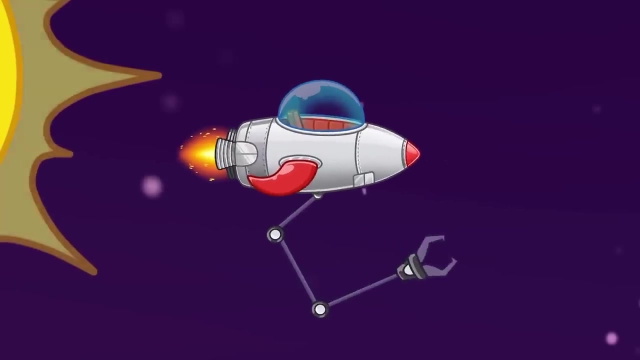 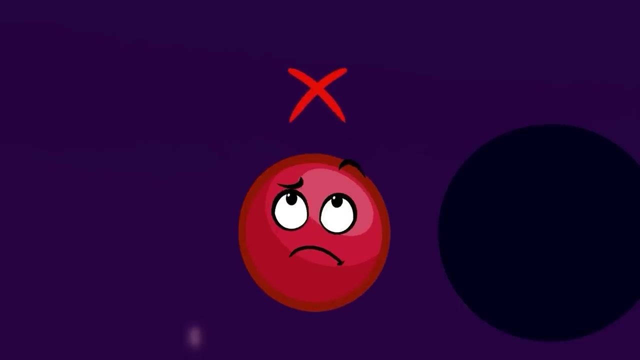 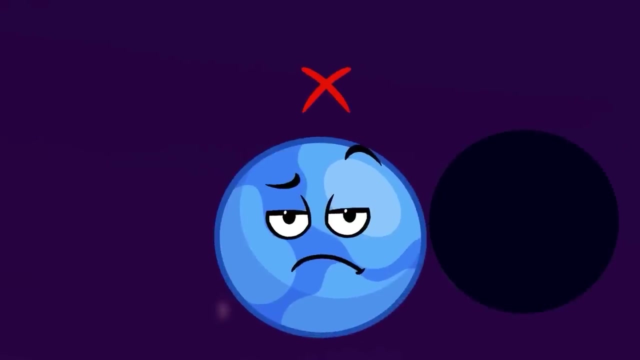 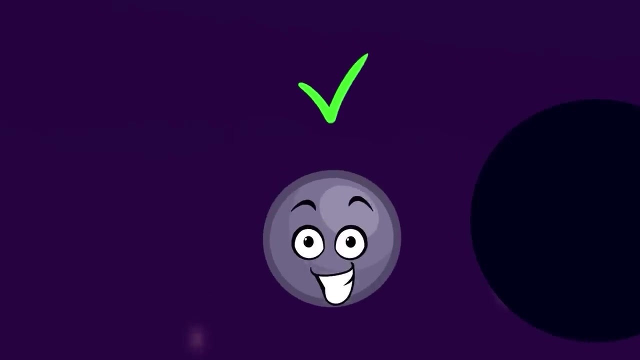 Pit has an idea. The feather will do the trick. Let's put them back in their proper place. That's not the right planet. Try again, Pit. Not that one either. This one looks right. This planet is… Mercury And this is…. 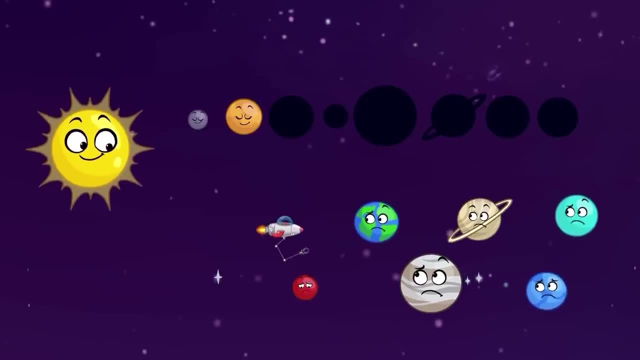 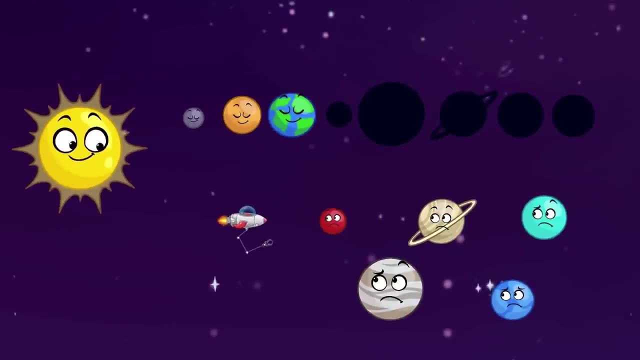 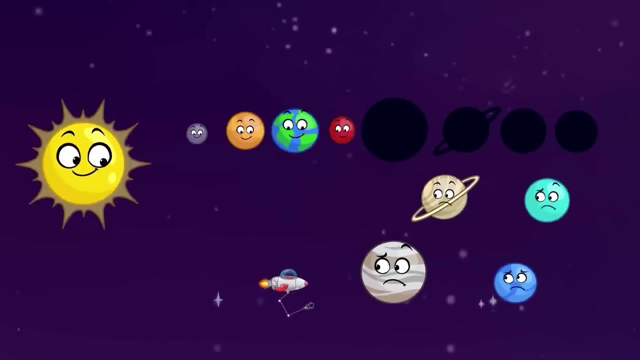 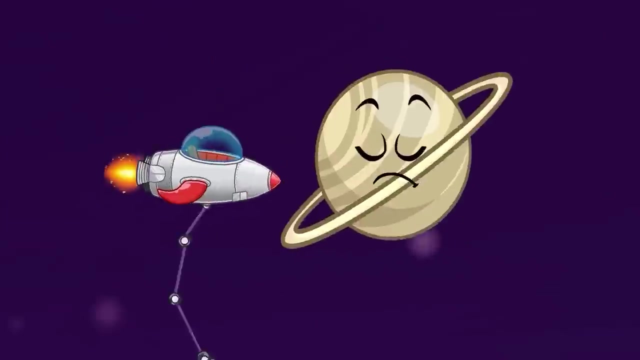 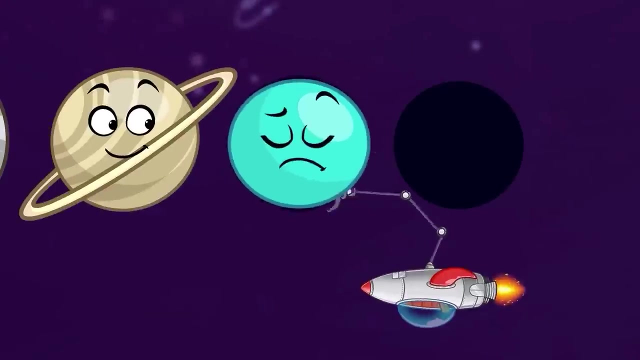 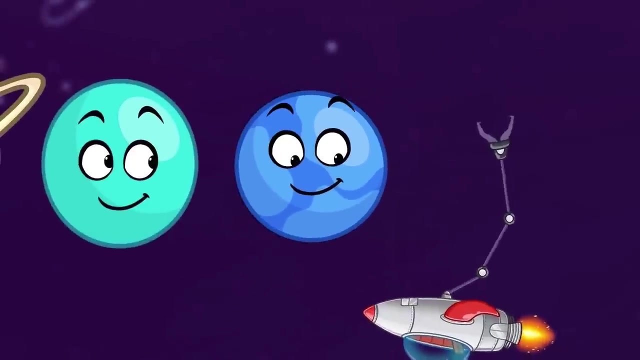 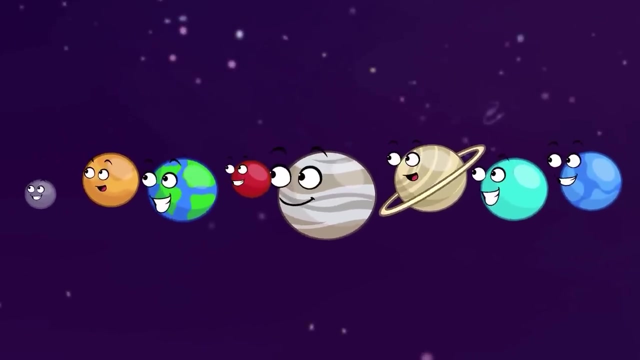 Venus, Next comes… Earth. Okay, Pit, Finish. the rest: Mars, Jupiter, Saturn, Keep going. Pit. Uranus, Uh-huh, And the last one is… Neptune. The planets are in the correct order. Pit, wake up. 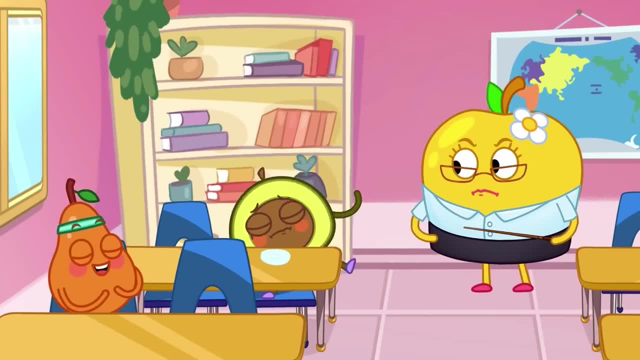 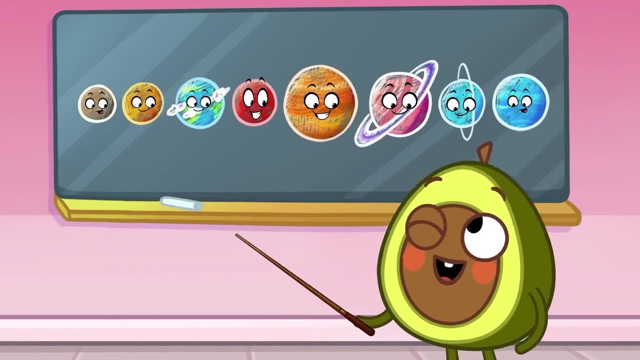 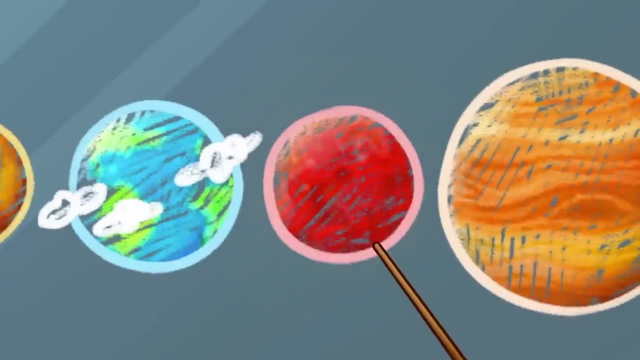 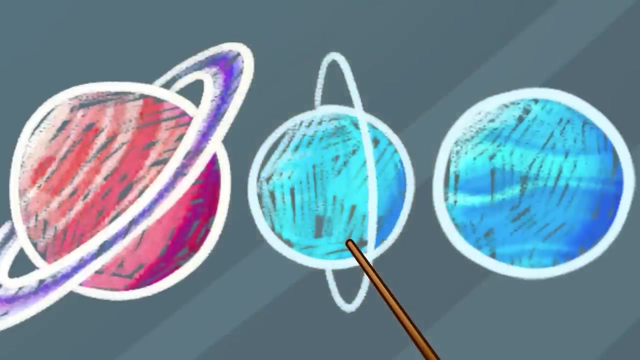 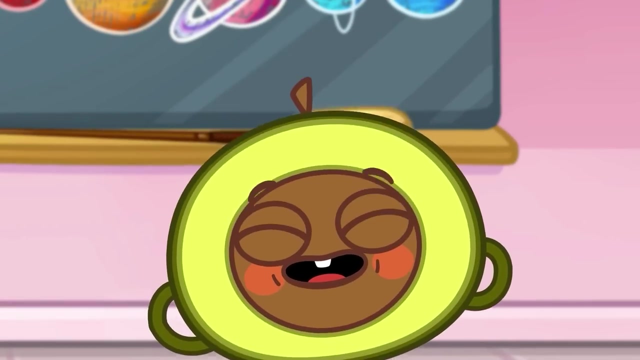 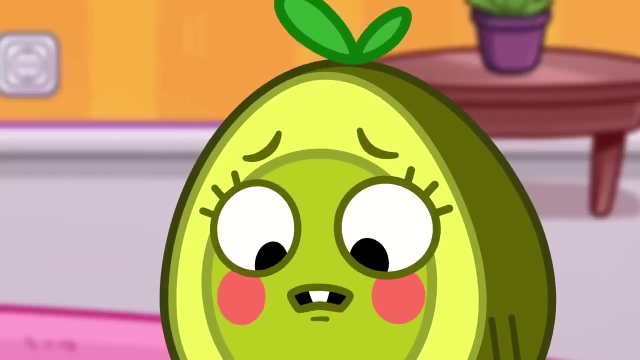 You were sleeping. Does Pit remember the planets? Mercury, Venus, Earth, Mars, Jupiter, Saturn, Uranus And Neptune? Pit remembered all the planets. Good job, Pit. Pit and Penny are playing with their toys. What's wrong, Penny? 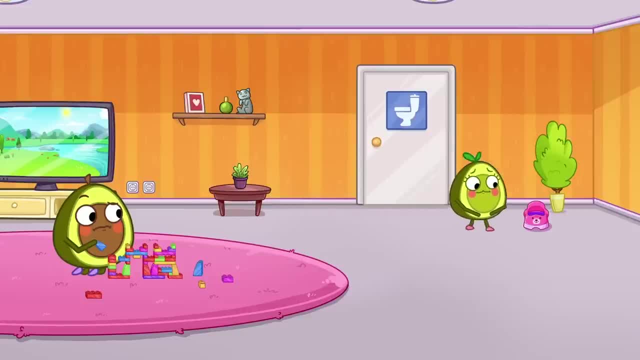 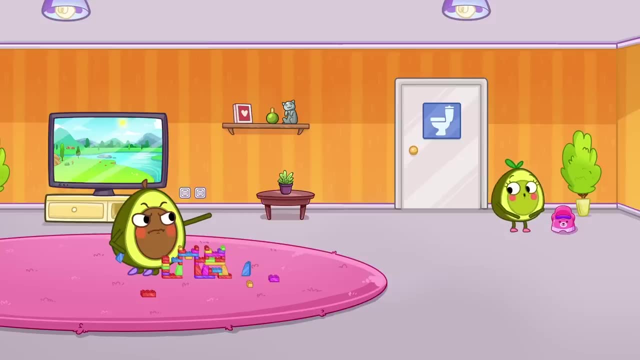 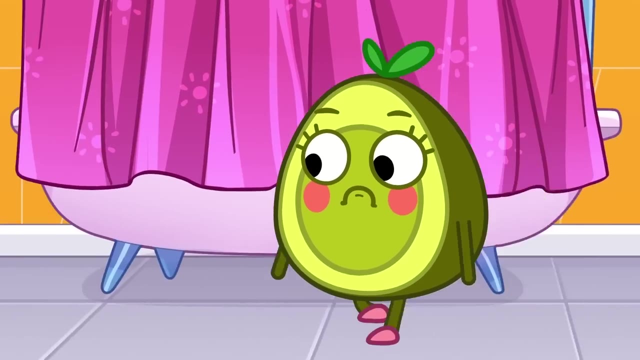 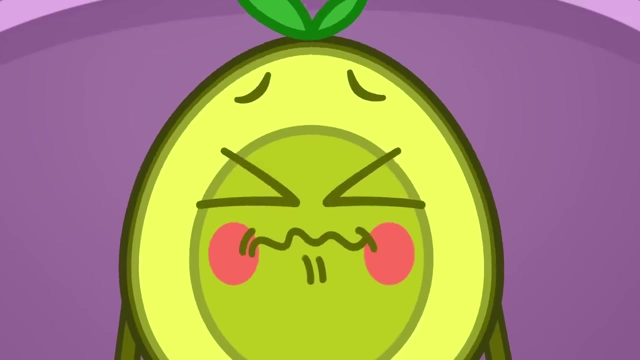 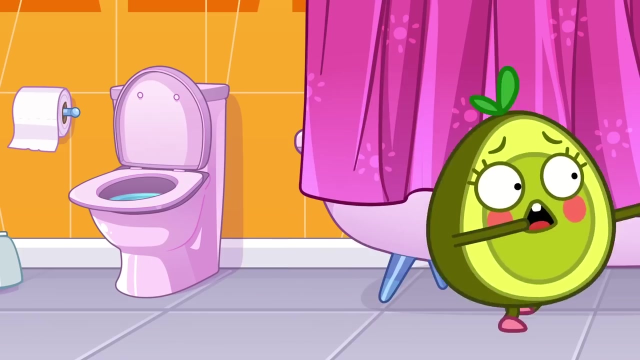 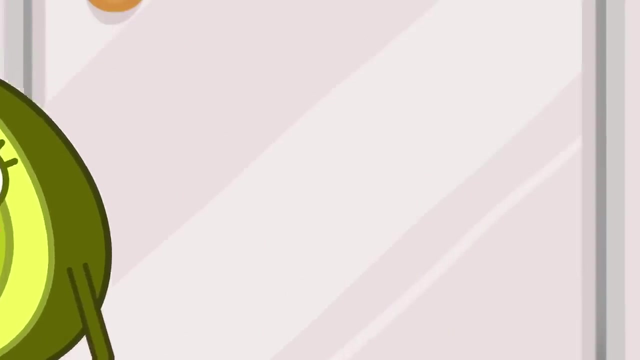 Penny needs to use the potty. This little one will work. Pit wants Penny to try using the big person potty. It's okay, Penny, You can do it. Poor Penny, She thinks she's too little for it. Penny decides to wait. 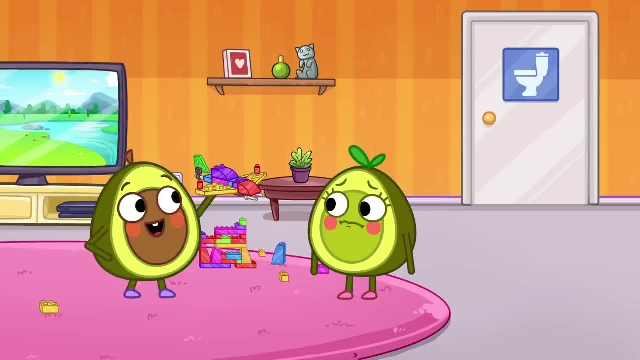 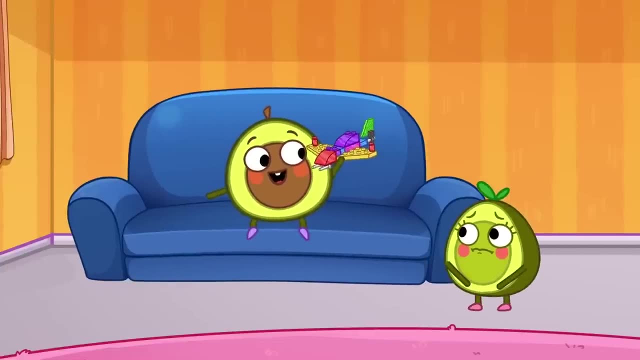 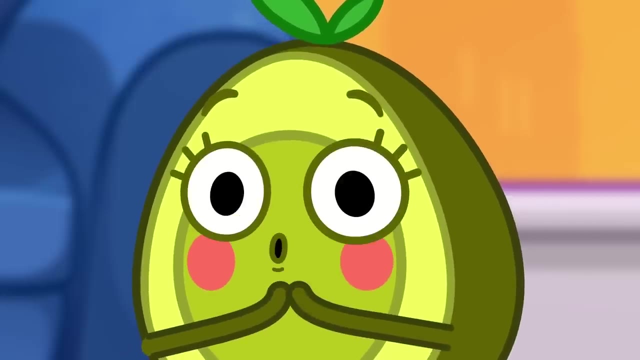 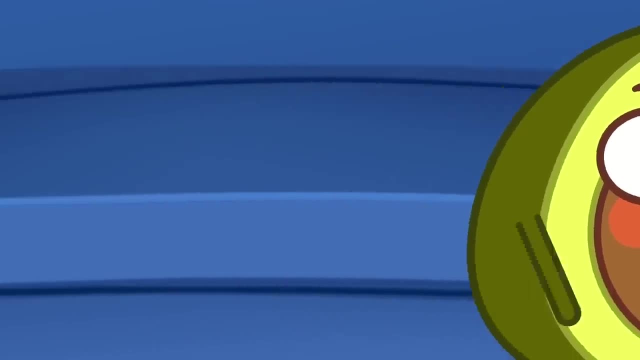 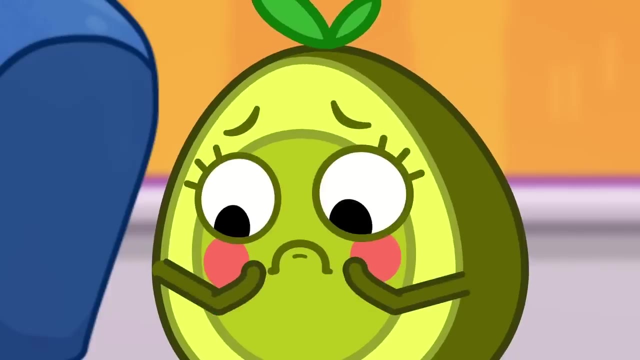 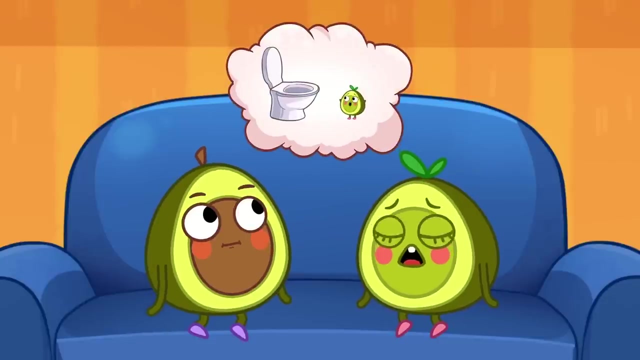 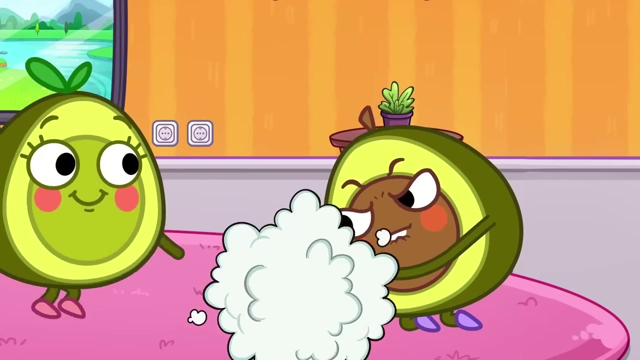 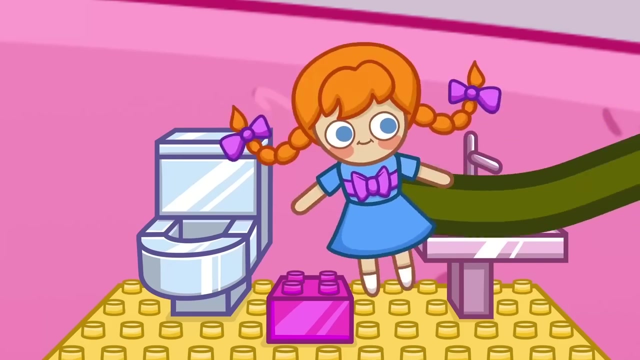 Look, you've made your sister cry. That's better. Pit is helping clean up the mess. What is Penny afraid of? Penny says she is too small for the big potty. Look, Pit made a tiny bathroom And he shows Penny what she needs to do. 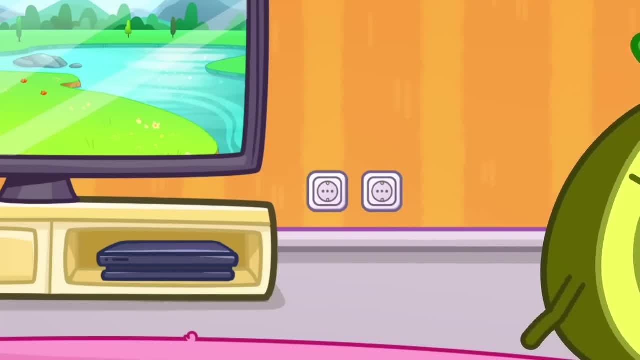 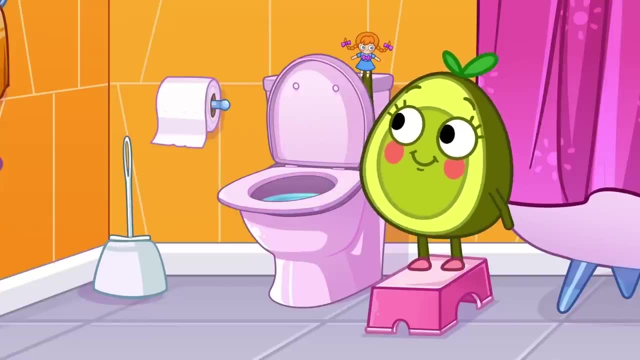 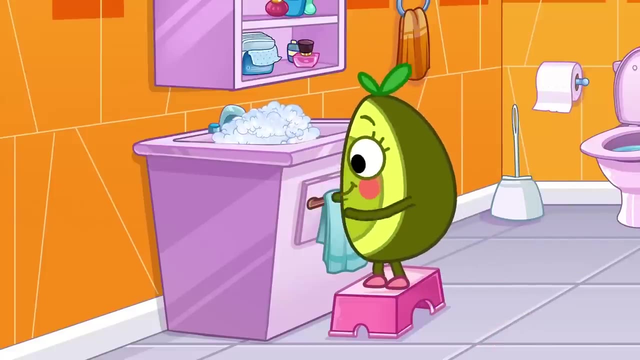 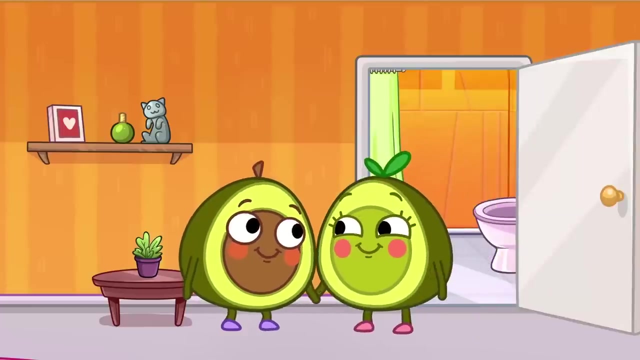 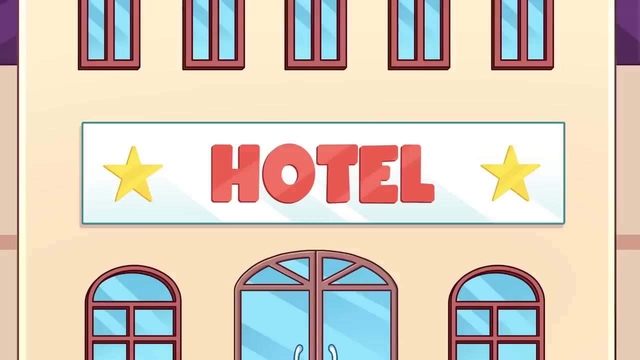 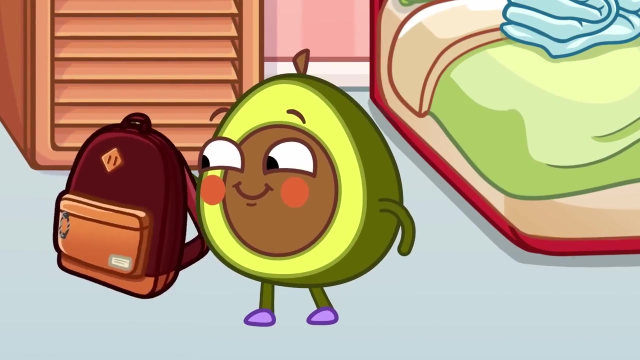 Penny is ready for another try. Well done, Thank you, Pit. Now Penny is ready to play. Pit and Penny are skiing at a hotel for the first time. Don't throw your bag, Pit, And don't jump on the bed. 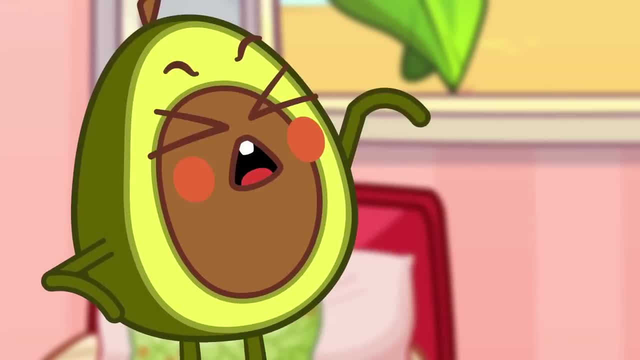 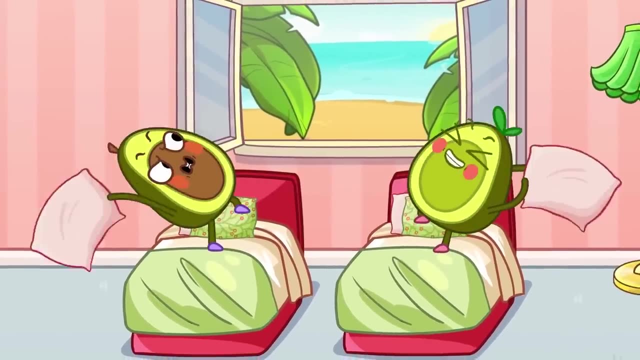 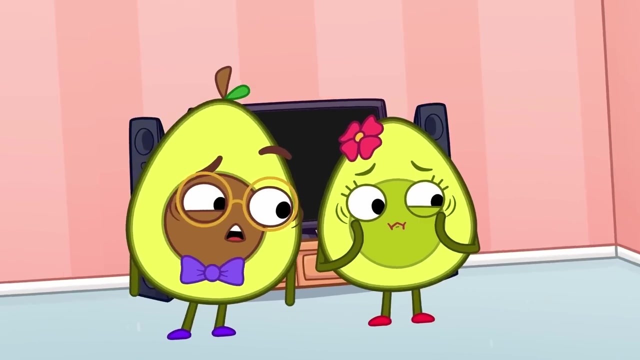 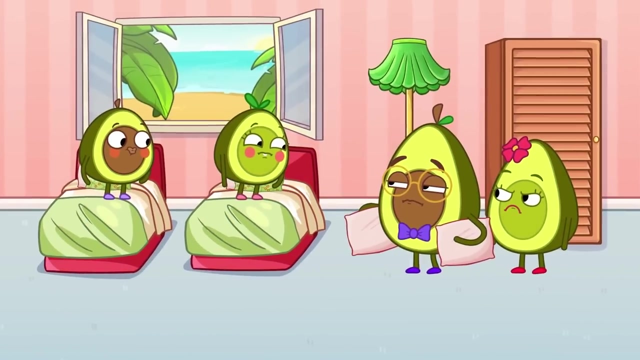 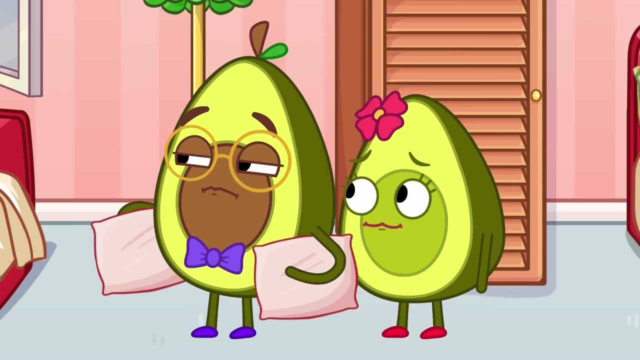 What's wrong? Pit, This bed will be mine. Now the kids are having a pillow fight. Daddy isn't very happy. Kids, Don't damage the property of the hotel. Mom and I have to go out. Wait for us here. 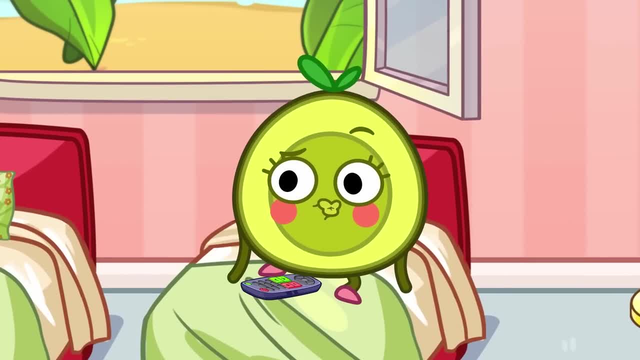 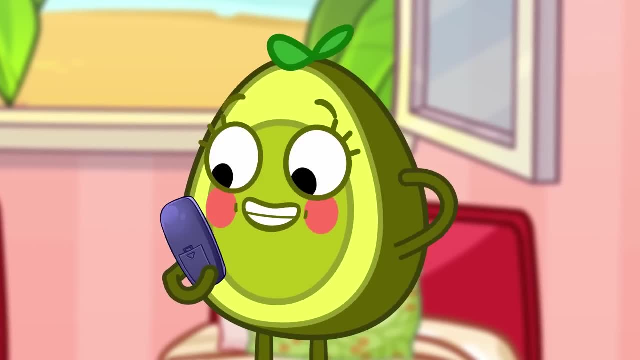 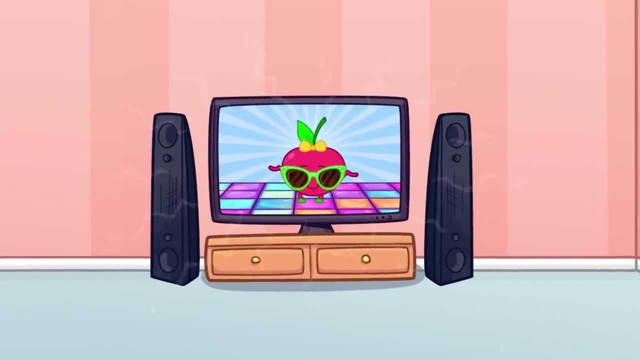 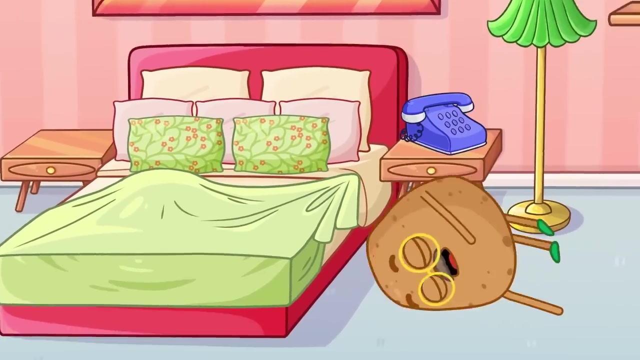 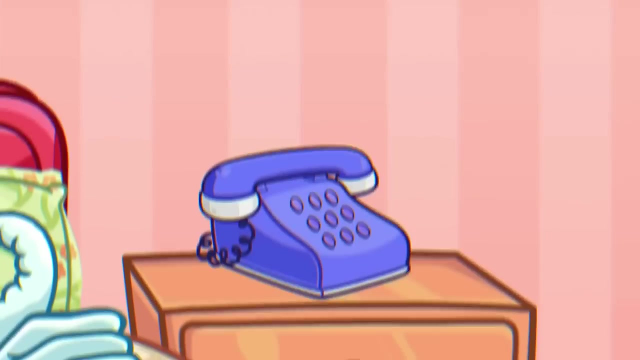 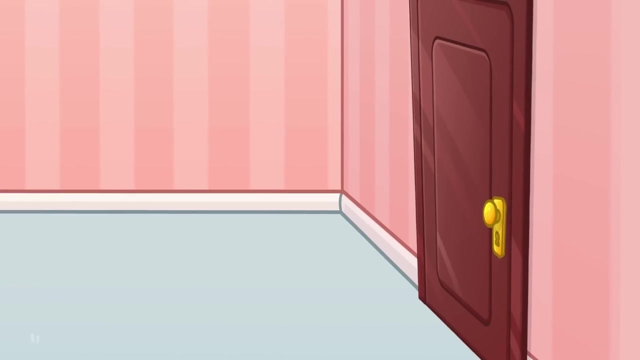 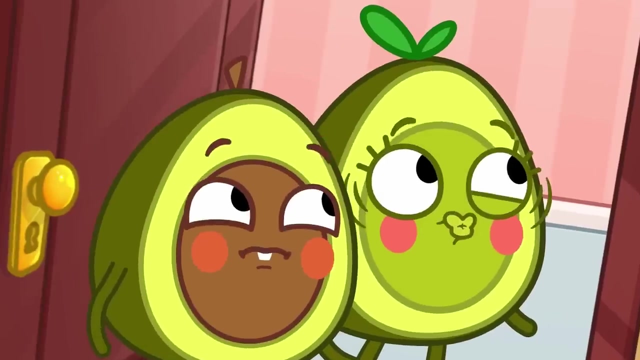 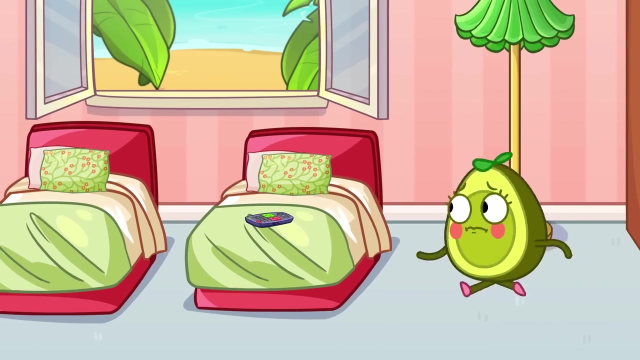 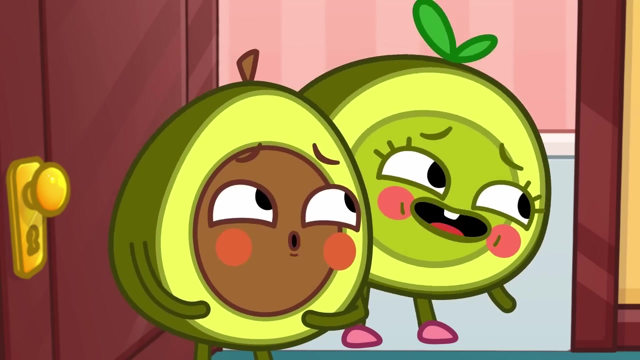 Maybe Pit and Penny can watch some TV. Penny, the volume is too high. Hey, look up, Mr Potato. Oh, Hmm, Someone's at the door. Kids, No noise in the hotel. It disturbs other guests. Yes, 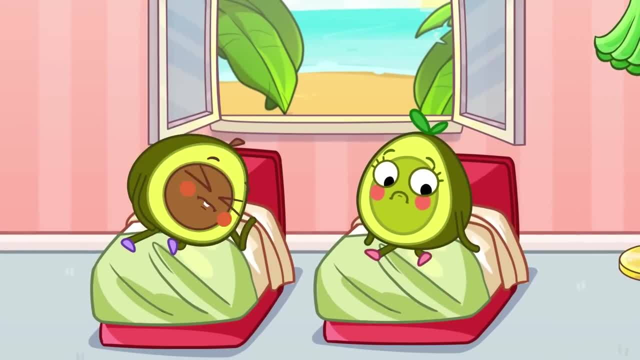 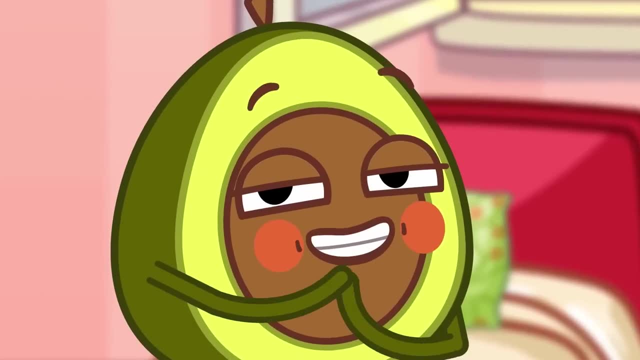 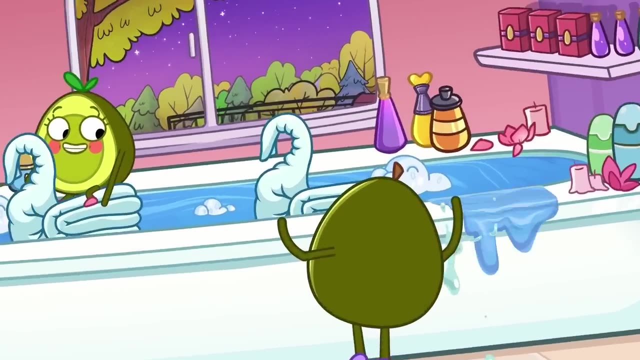 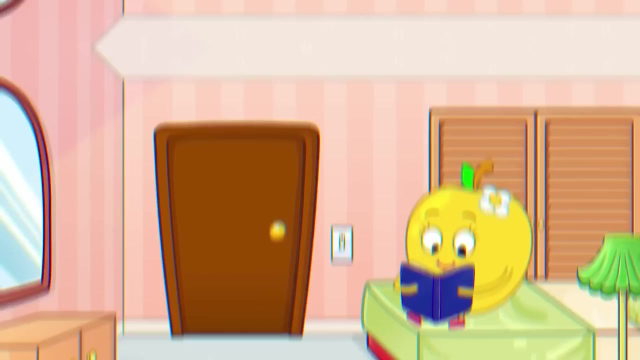 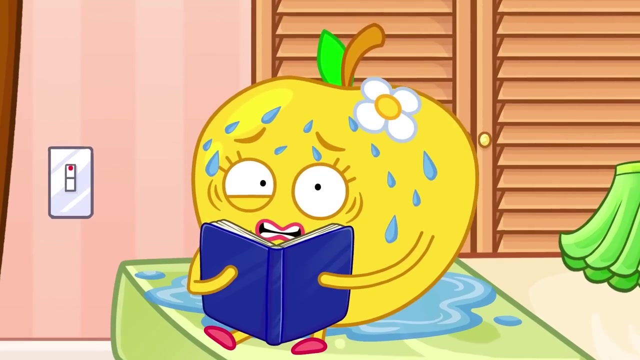 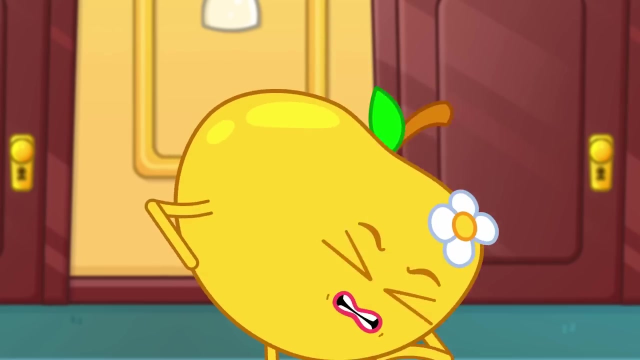 Please, Sorry, Now what can Pit and Penny do? Penny has an idea. Oh, Now they're playing in the bath. And water is getting everywhere. Oh, Oh, Oh, Oh, Oh, Poor Miss Apple, You are flooding my room. 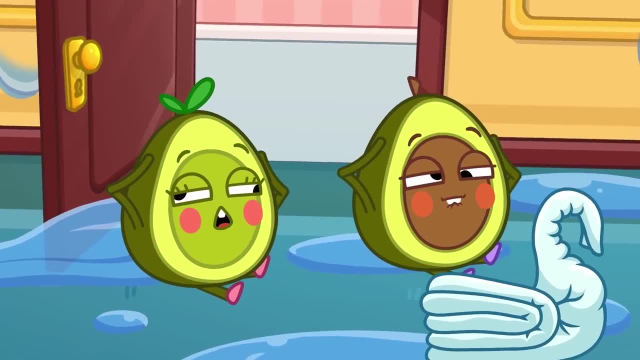 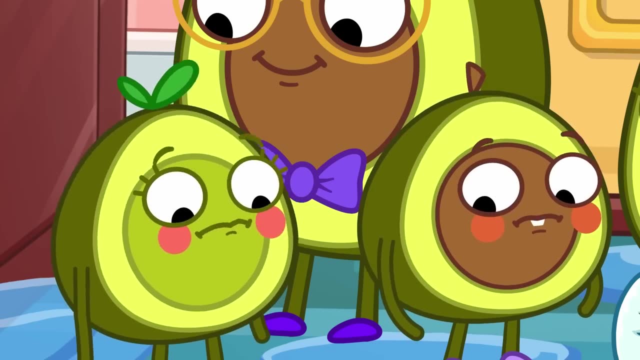 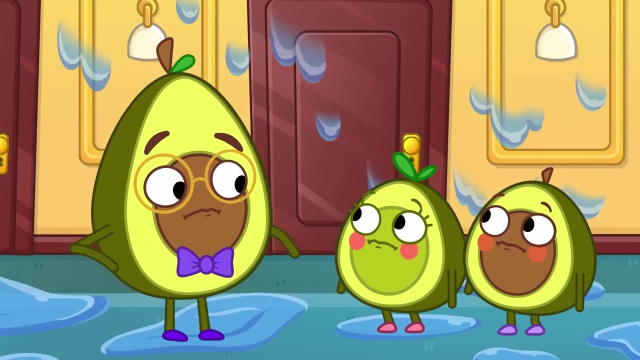 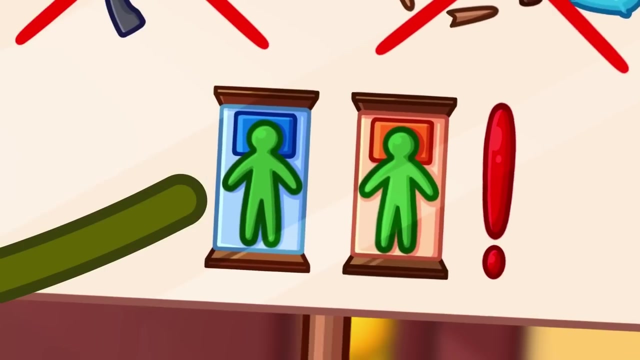 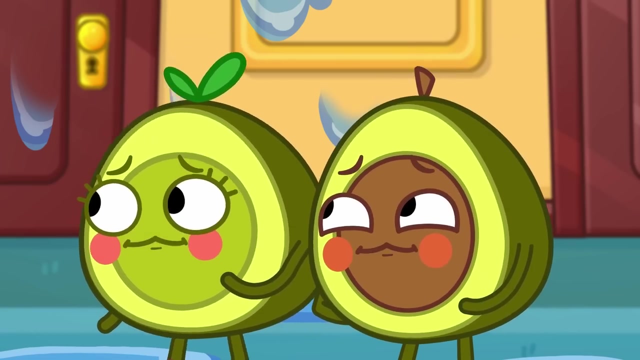 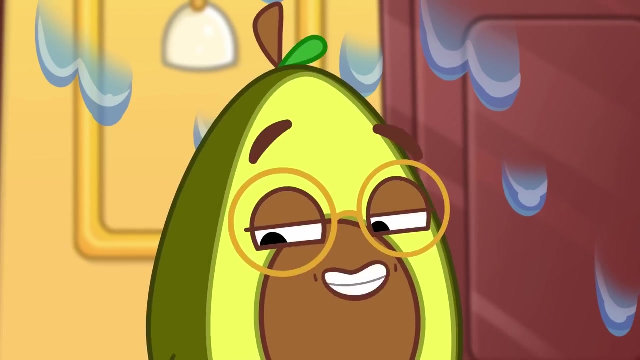 What a terrible mess. Kids, Are you okay? I need to remind you of the rules again. No loud noises. Don't play on furniture, Respect others, Remember these rules and everything will be fine. Yes, sorry, Now that you know them, Let's go to the restaurant. 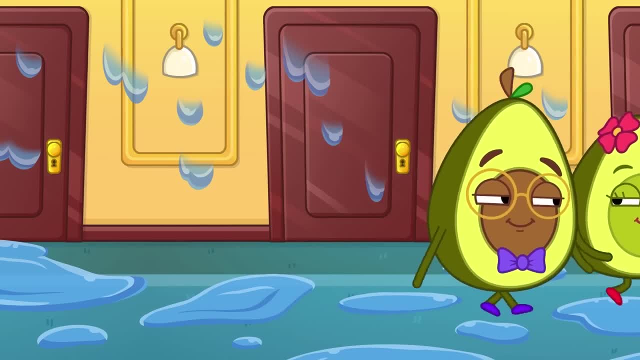 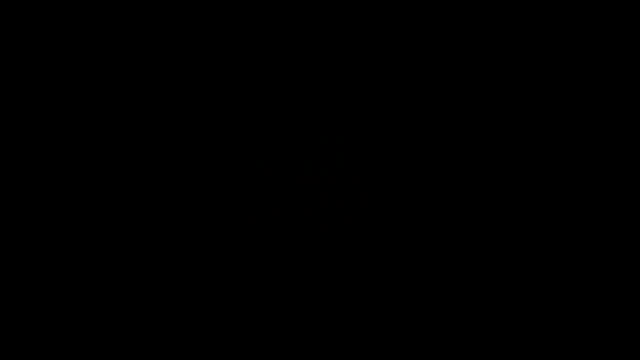 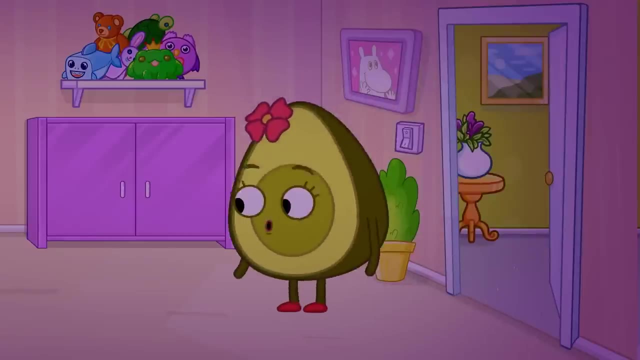 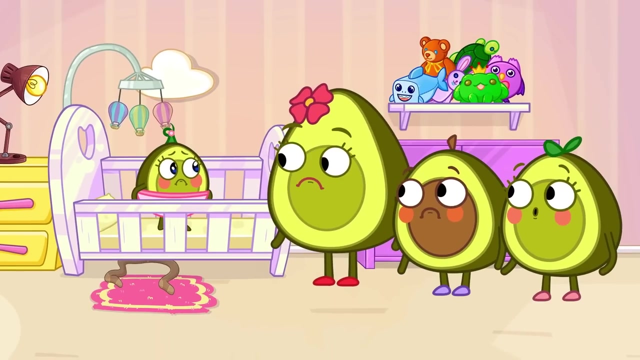 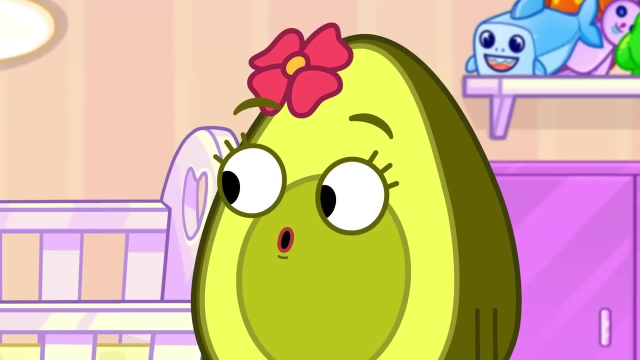 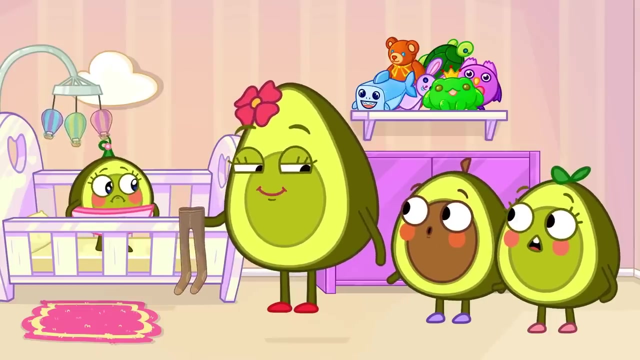 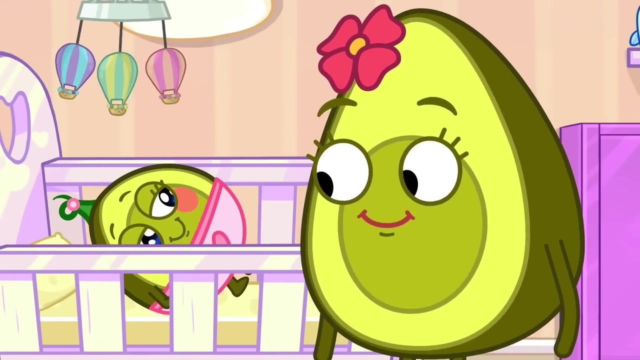 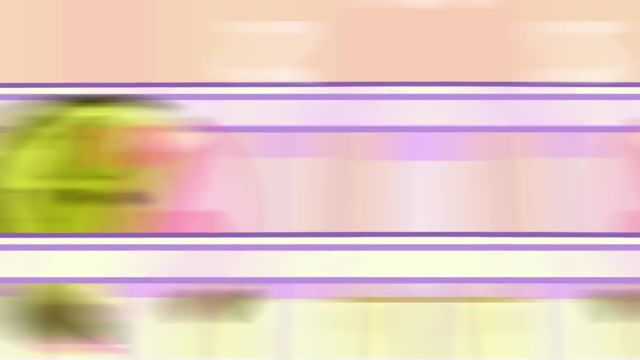 I hope you have fun. Strawberry will clean up the mess. Something is under the crib. What's happened? Baby's afraid There's a monster down there. Someone has forgotten That site's here. See, Monsters aren't real. You have nothing to fear. Night-night baby. 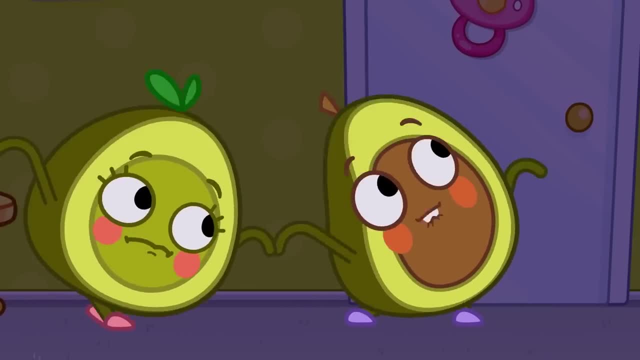 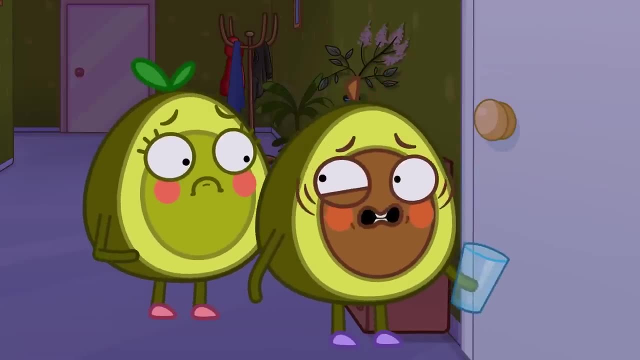 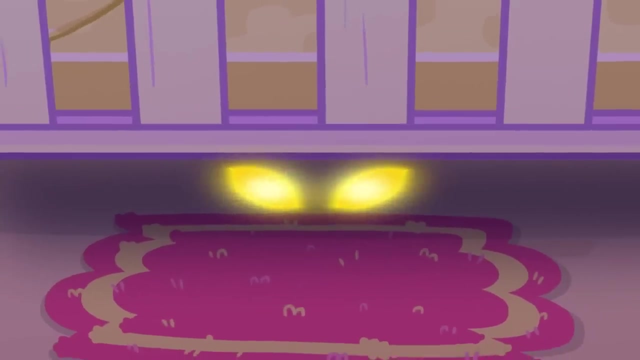 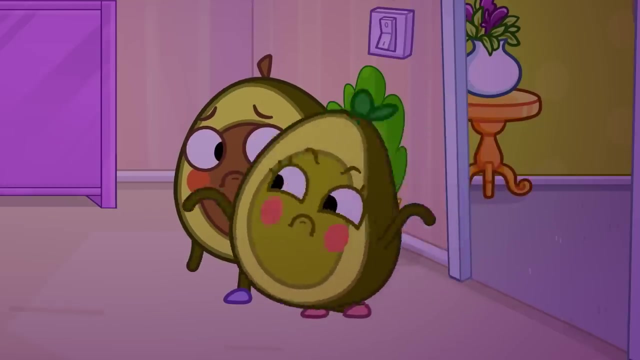 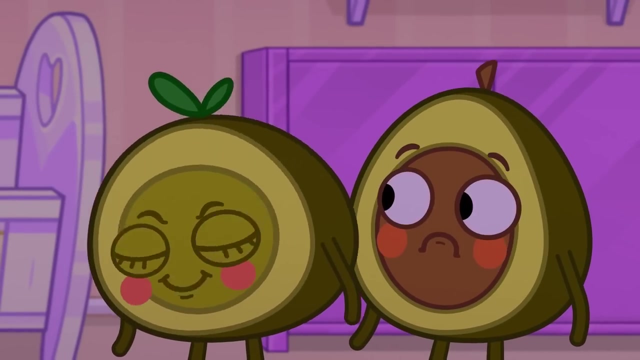 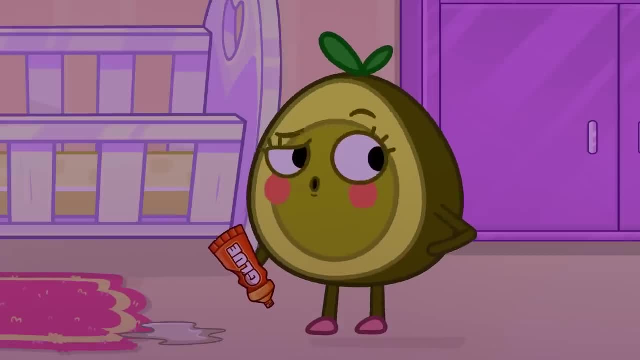 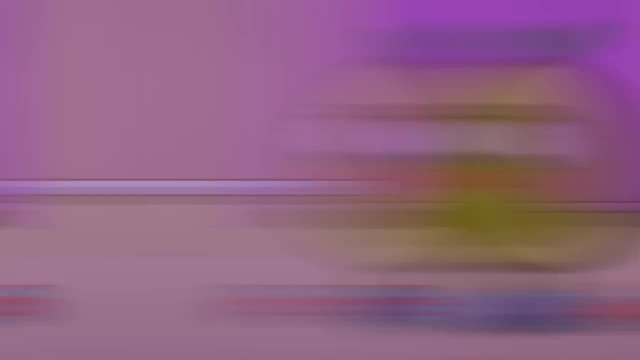 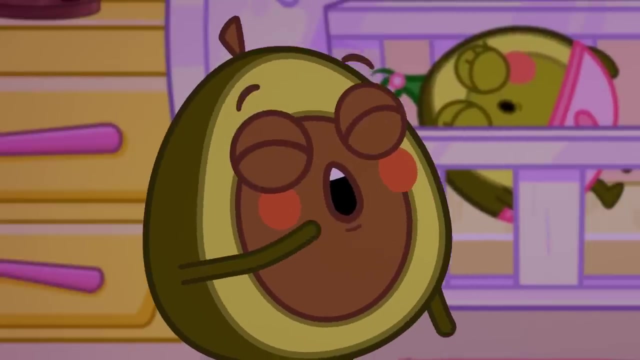 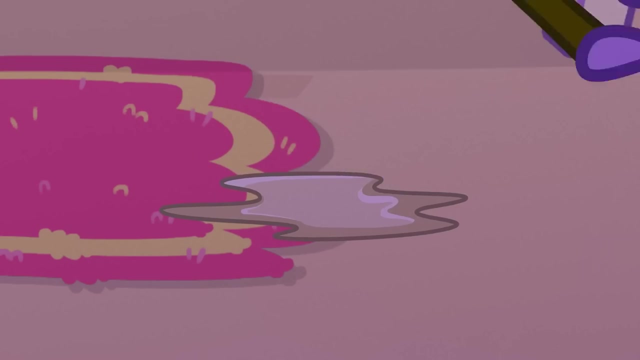 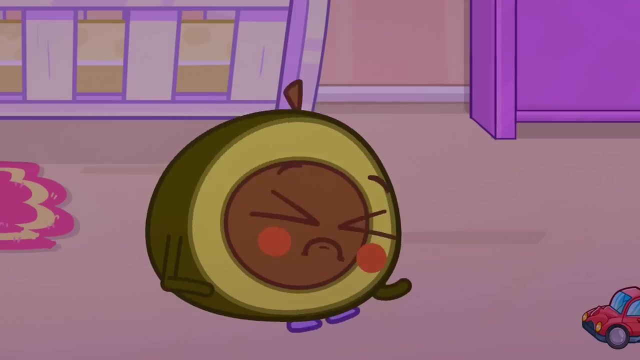 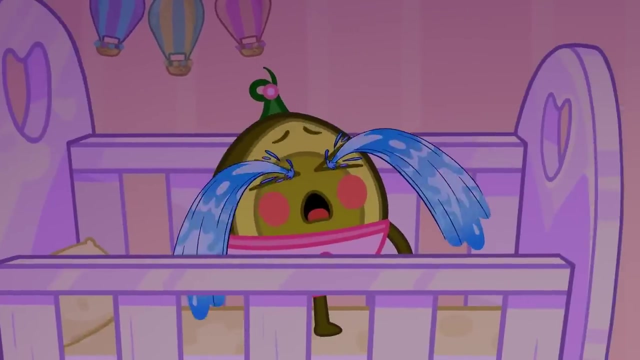 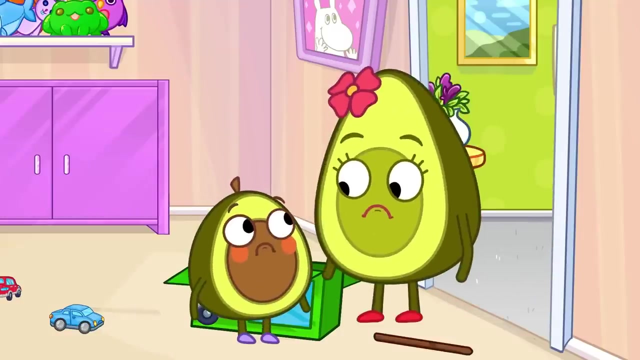 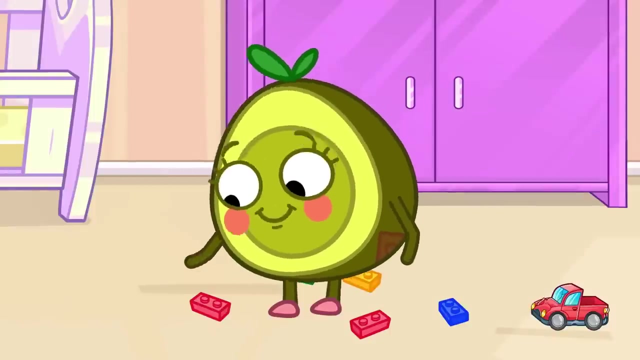 Maybe you could set up a monster trap. This will stop the monster. The robot can stand guard And the monster will be trapped in the box. Let's go to bed. Oops, you trapped Pit instead And you woke up, Baby. What's happened here? The kid saw a monster. 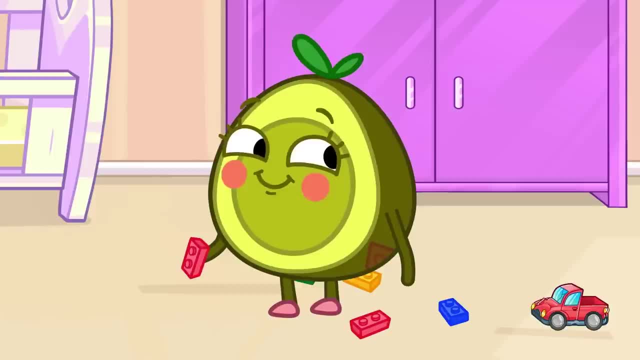 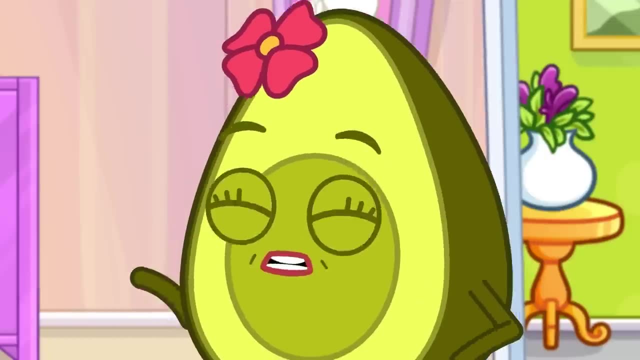 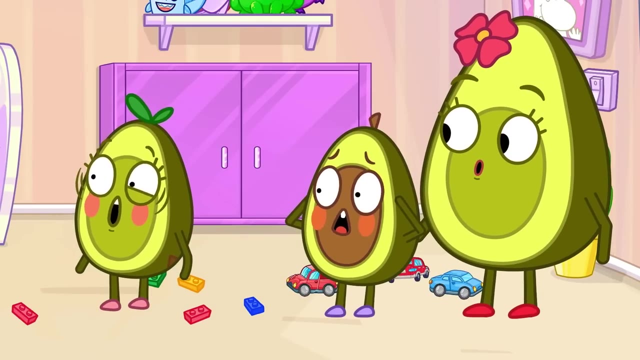 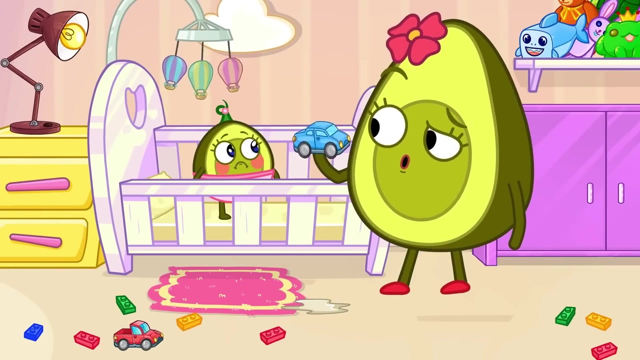 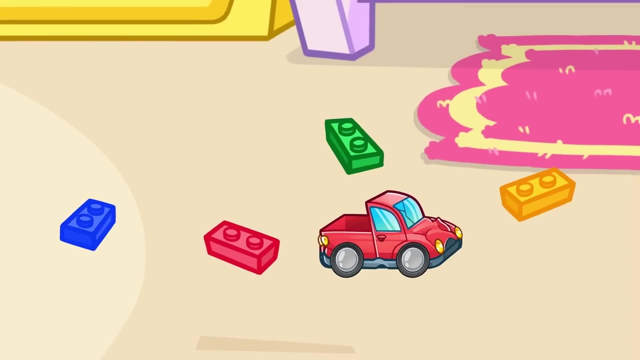 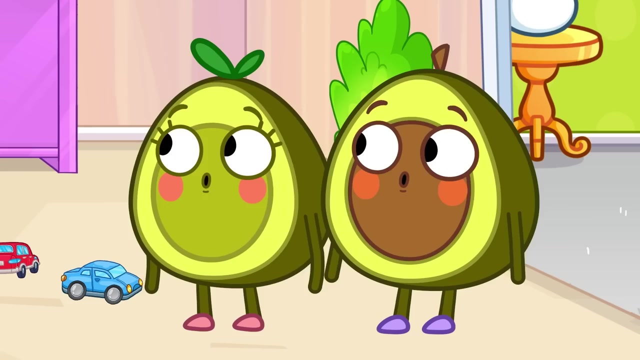 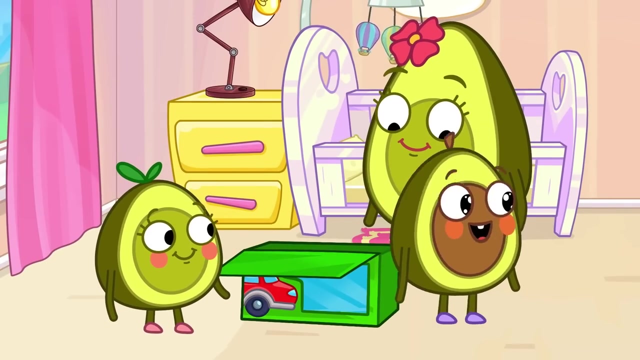 It seems this is the monster That bit me. Sure monsters don't exist there. Then what is under the crib? It's Pit's toy, My car. Look at this mess. You should put your toys In the box, kids, The room is nice and clean. 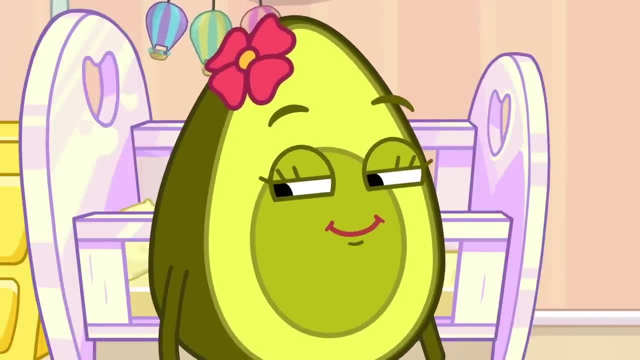 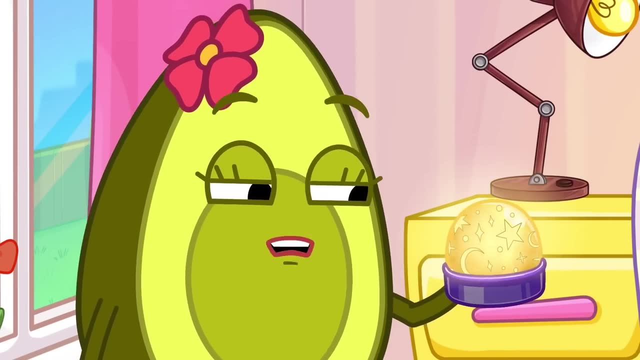 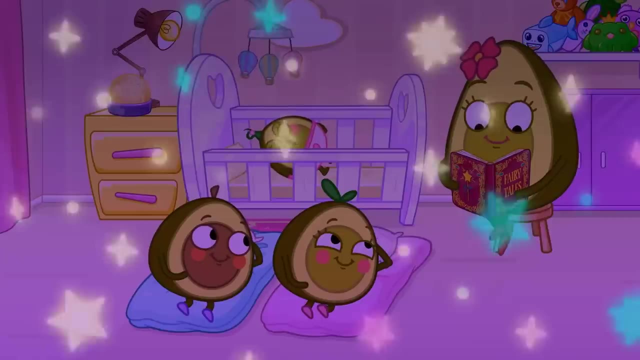 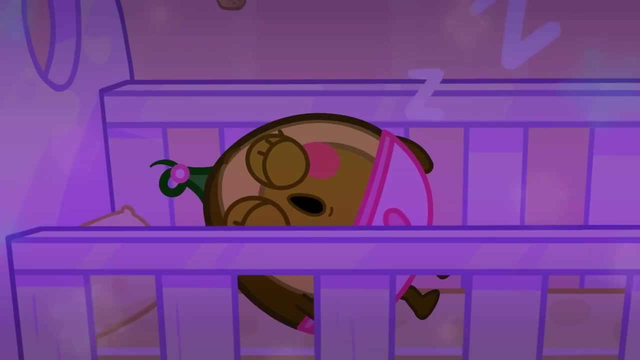 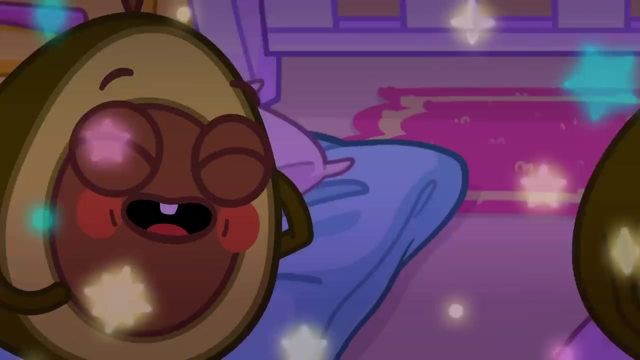 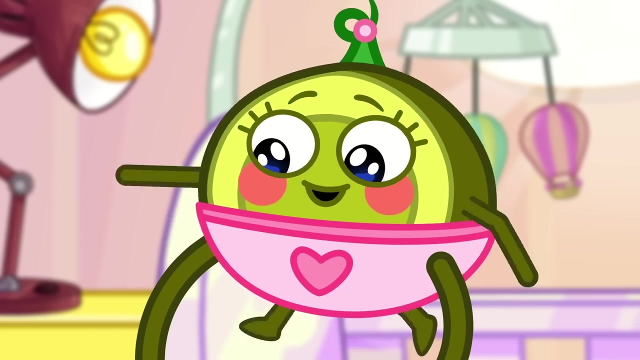 Now nothing will scare you. Oh, What is the night light for? This light will help you sleep peacefully, And they lived happily ever after Shh Baby's sleeping, And so are Pit and Penny, Nighty-night everyone. It's time to wake Baby up. 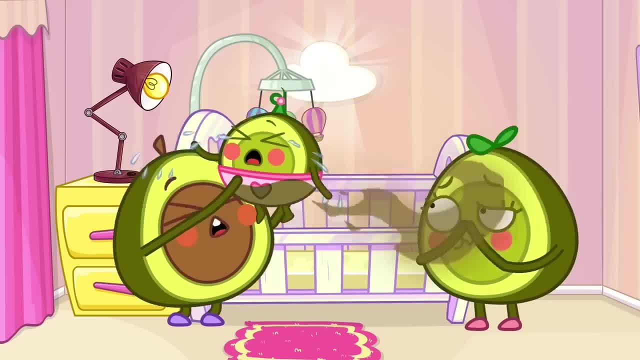 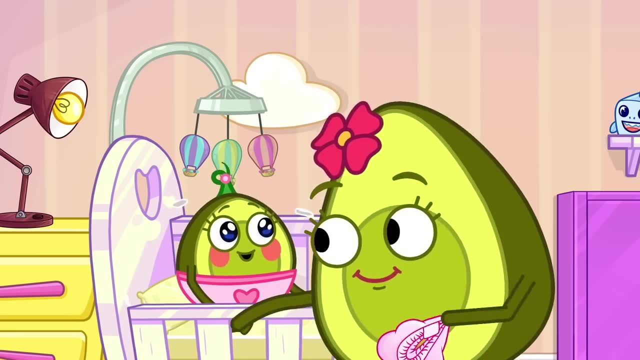 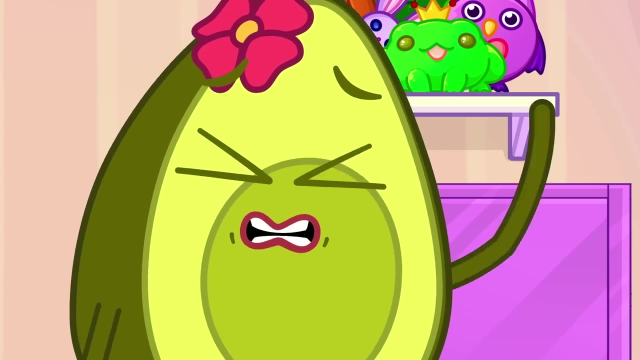 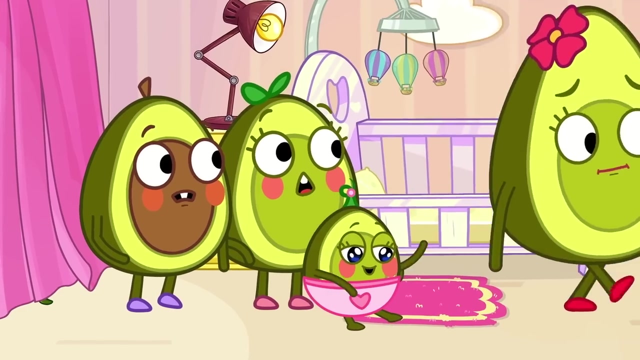 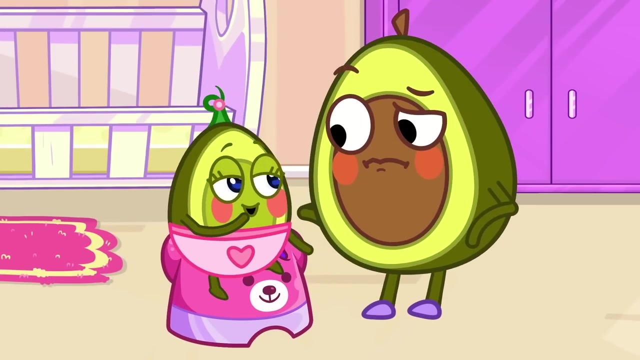 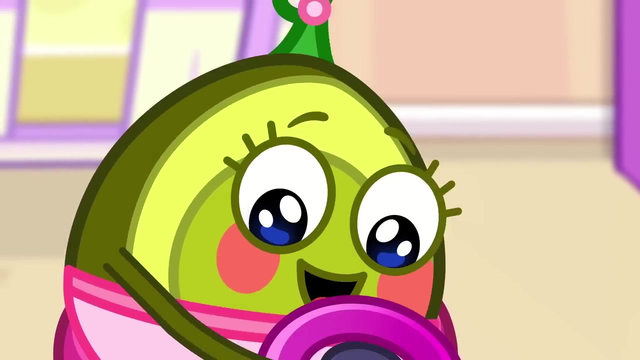 But Baby made us stinky. Don't worry, Mommy will change her. But changing diapers is hard work. How can Pit and Penny help? Baby needs potty training. Baby's never used a potty before. She thinks it's a toy. Pit will try to explain. 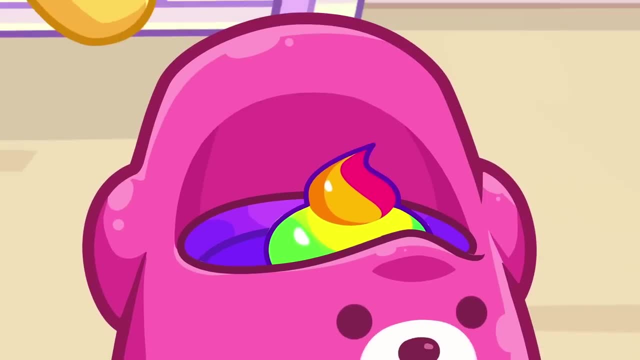 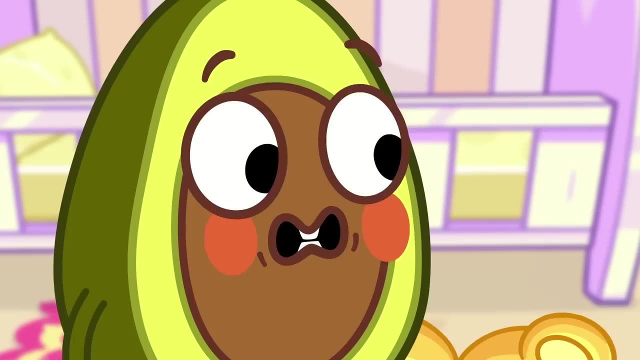 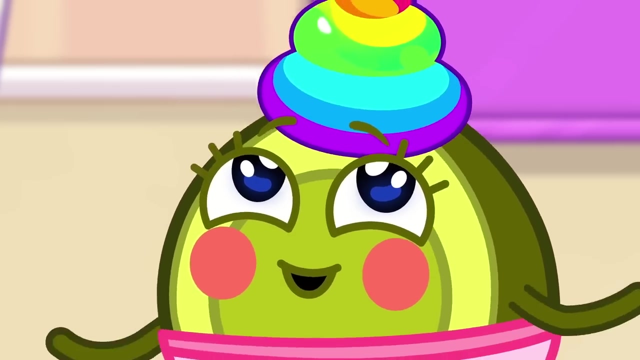 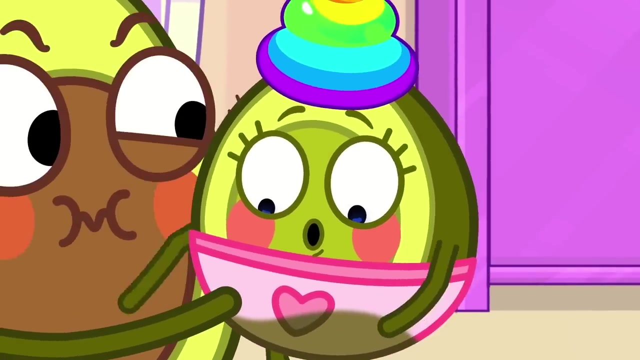 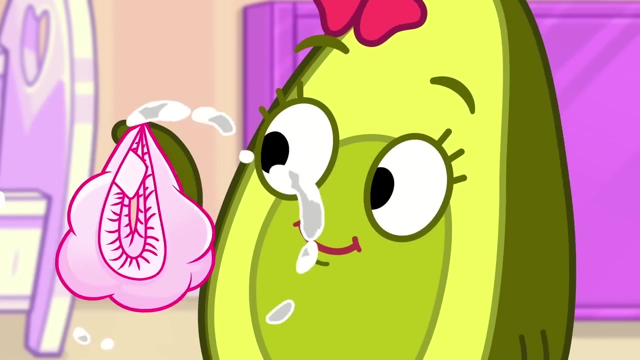 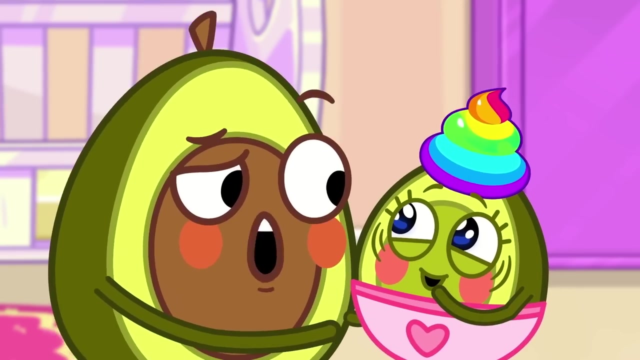 See, This is where the poop goes. Baby thinks the potty is a hat. Over here, Suvarnabhumi, Pit wants Baby to keep trying. Mommy will change this dirty diaper. Mommy has available, necessary, finished. slowly Wait for me, Baby says. 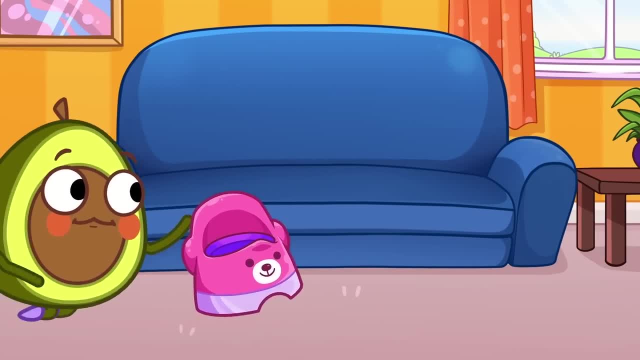 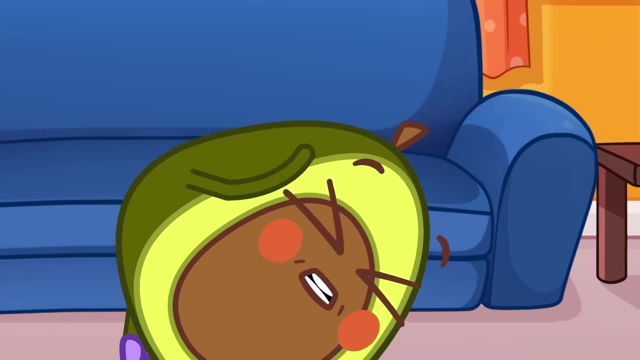 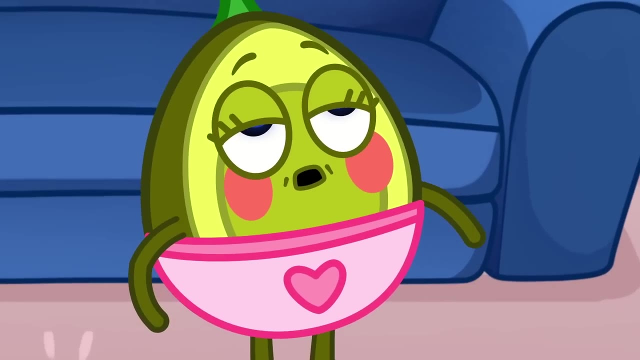 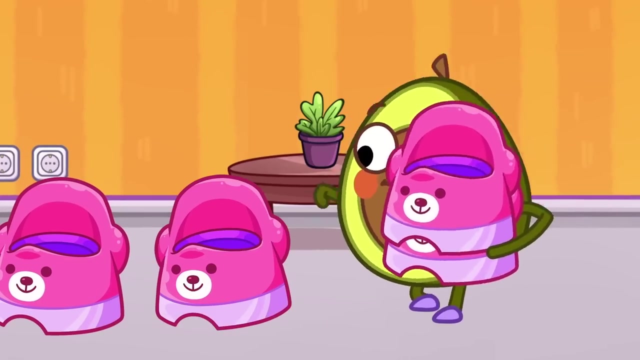 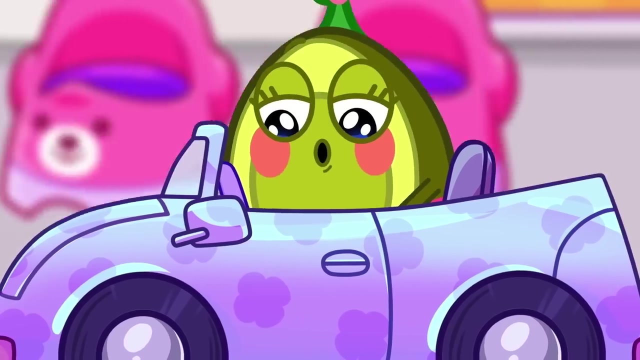 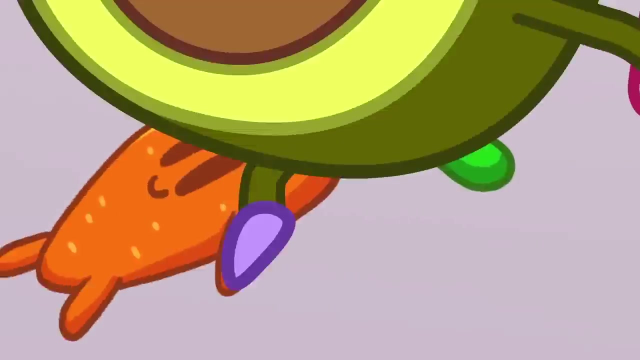 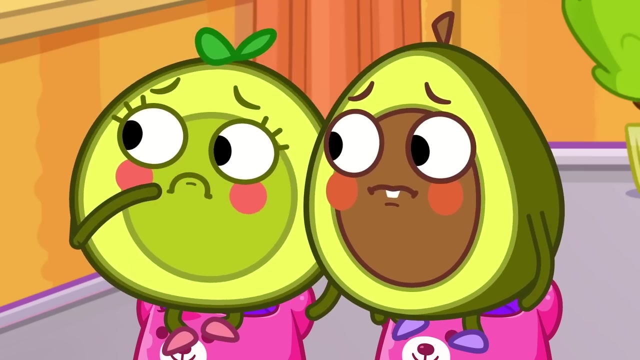 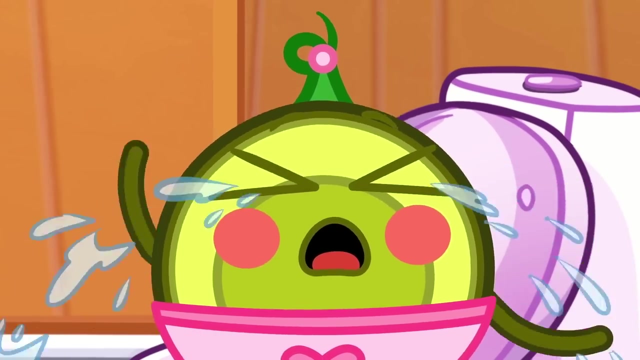 Pees. They'll follow her with a potty. They'll push the potty in place. They'll put potties everywhere. Maybe she doesn't like potties. They'll even try the big toilet, But it's too scary. 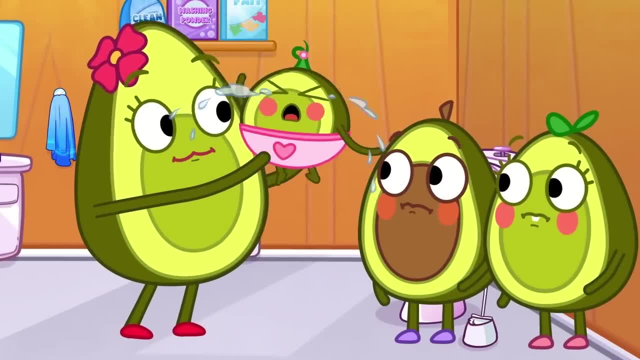 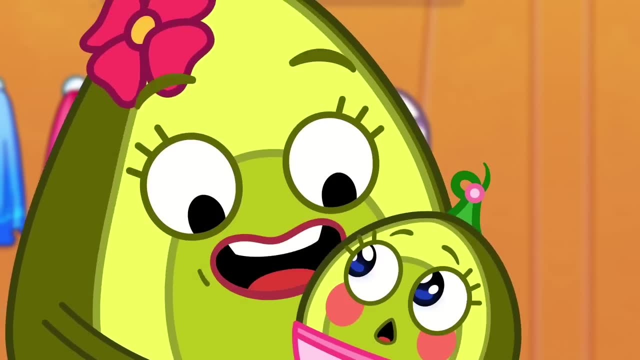 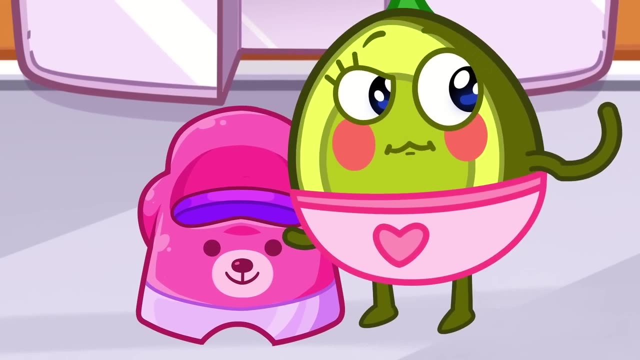 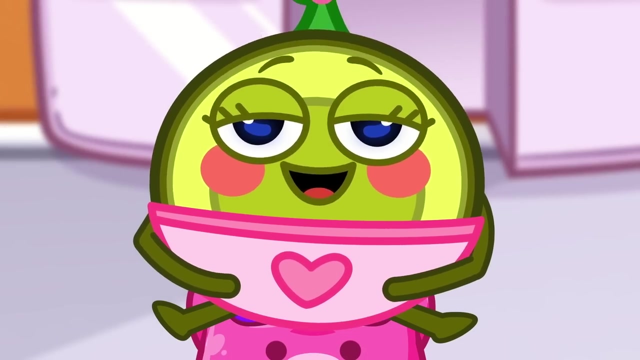 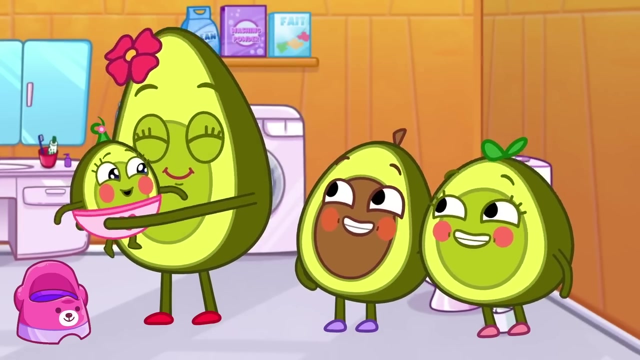 Mommy, Baby won't stop crying. We wanted to toilet train her. She's still too small for your potty. Everything has its time. Yay, Baby's doing it. Good job, kids. Penny lost one of her teeth. 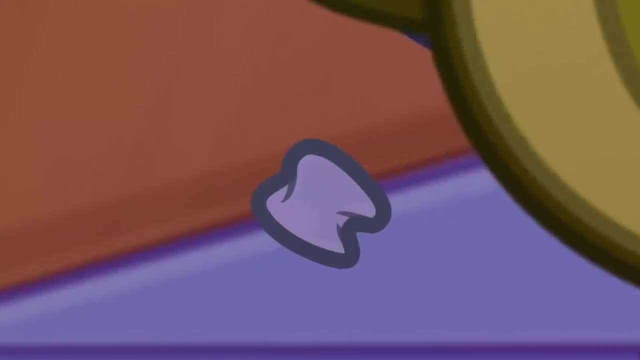 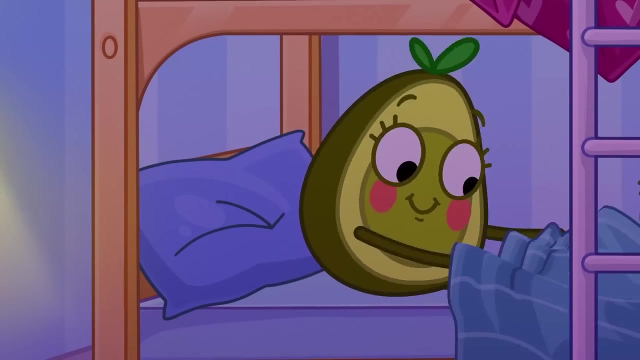 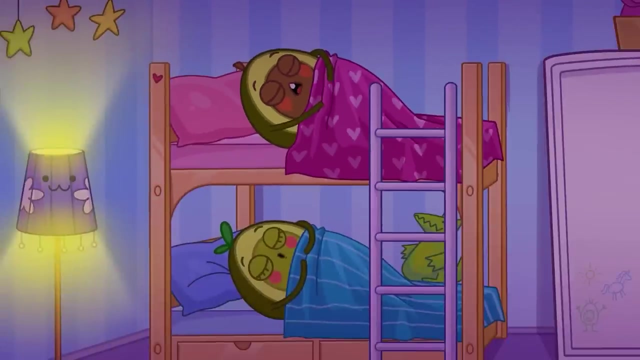 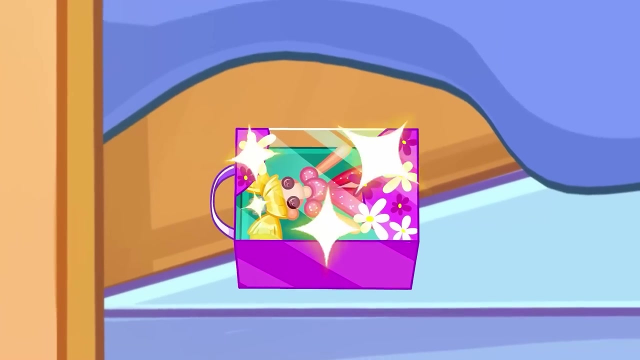 She'll put it under the pillow for the tooth fairy. Maybe she'll get a doll. Fairies don't exist, Are you sure? Pit, The tooth fairy is already here? A gift from the tooth fairy. Penny got the doll she wanted. 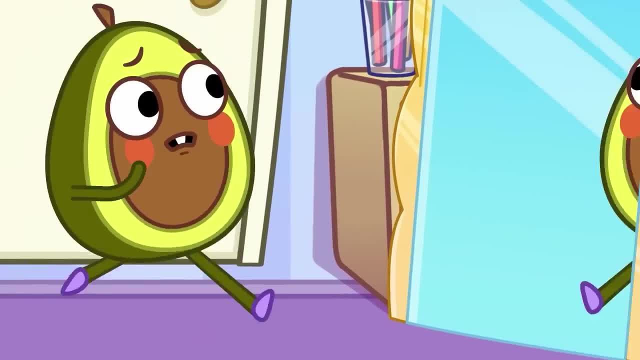 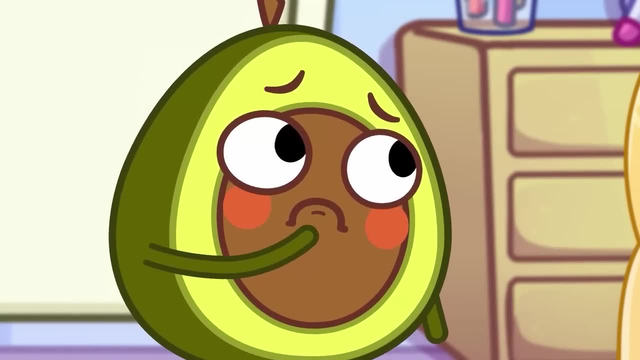 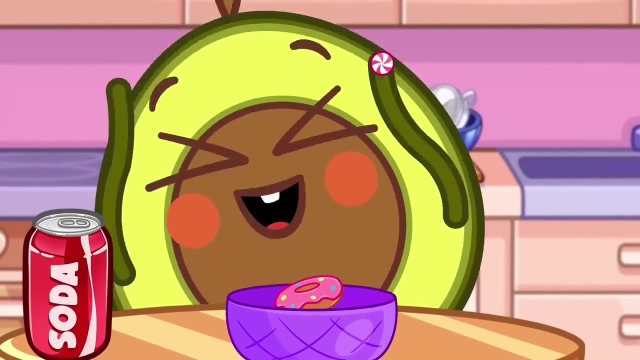 It can't be true. Now, Pit hopes he has a loose tooth, But he doesn't. He thinks eating lots of sweets will loosen a tooth, But it seems like he'll have to go to the toilet. We promised to make the doll. 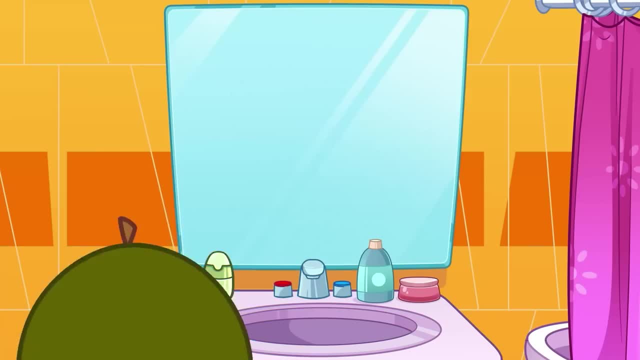 Did you hear that? But there's no stick inside the doll, It's gone. We're done. now She's got to wait to show us Pit. We'll wait until after the end And then we'll clean her up And when the job done we'll go home. 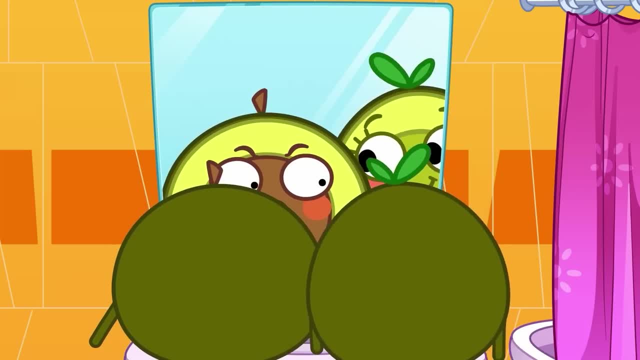 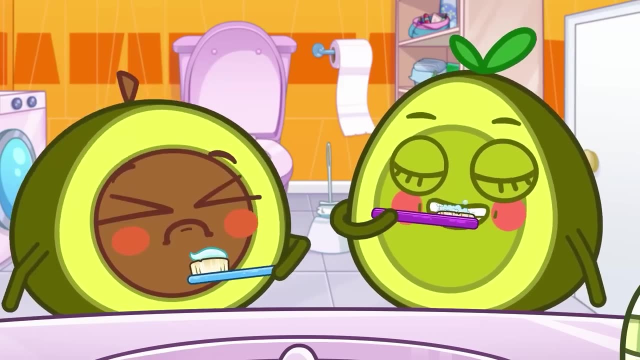 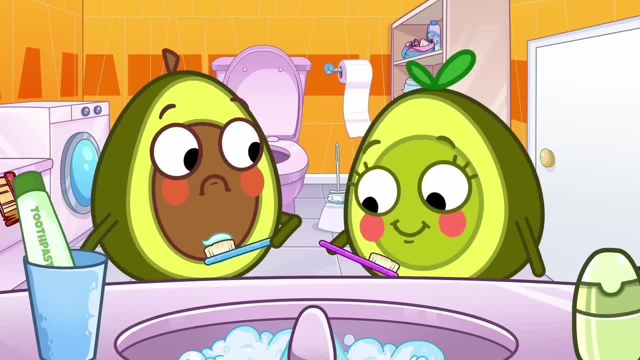 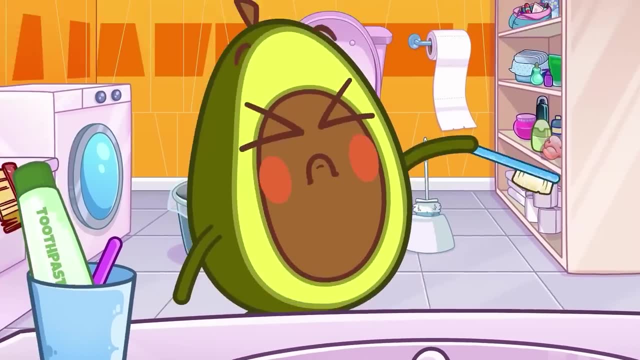 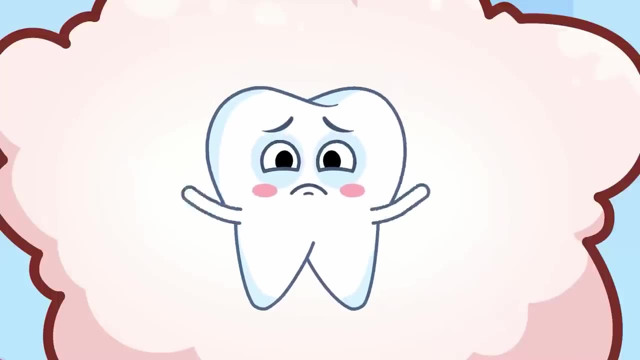 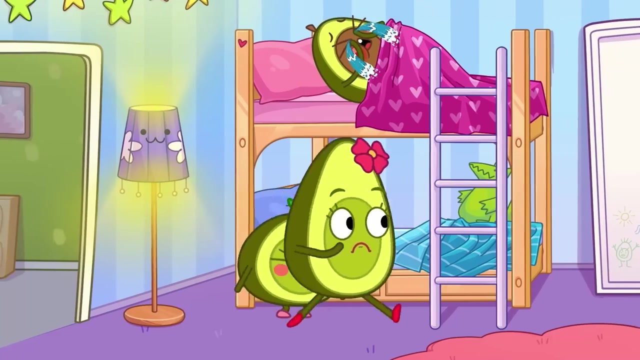 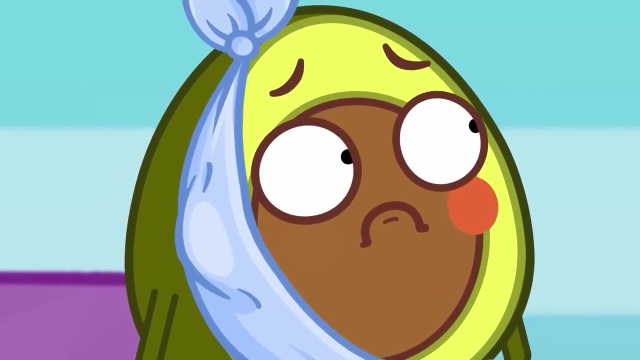 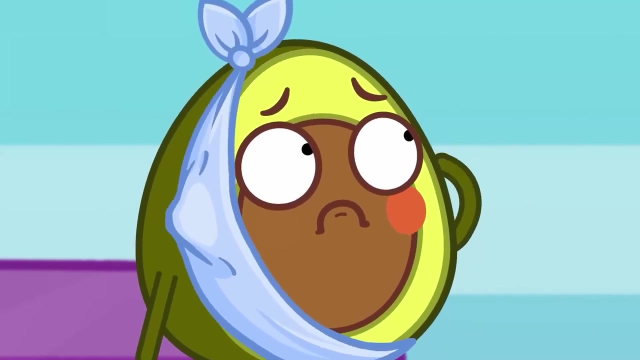 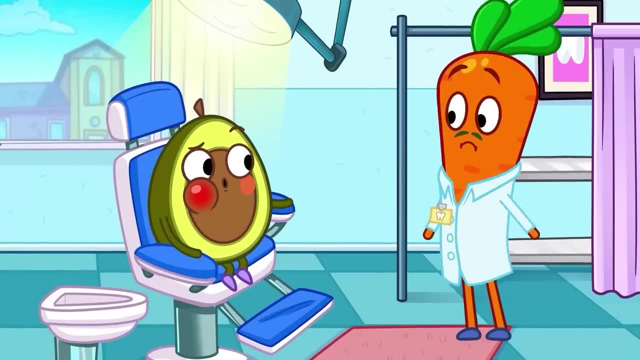 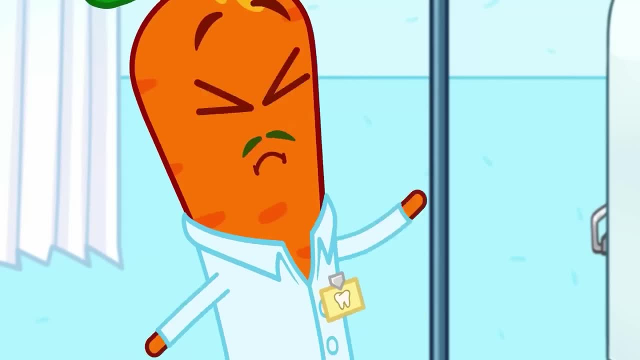 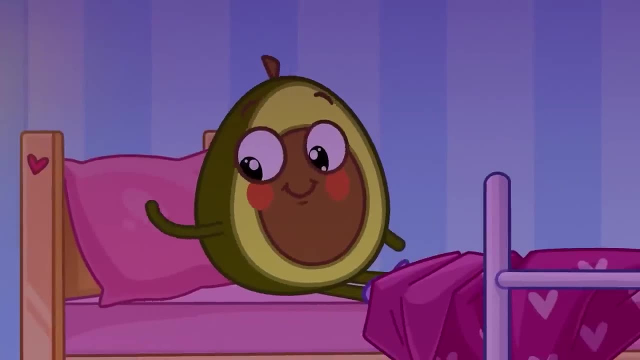 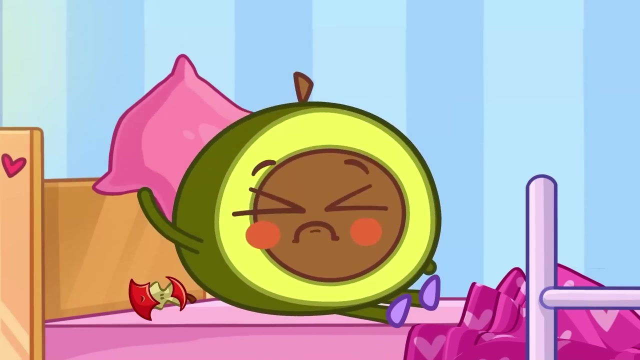 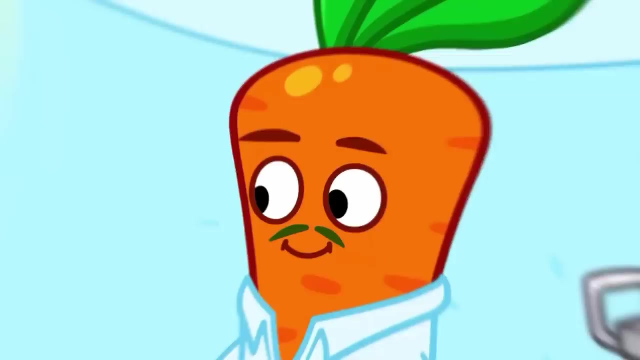 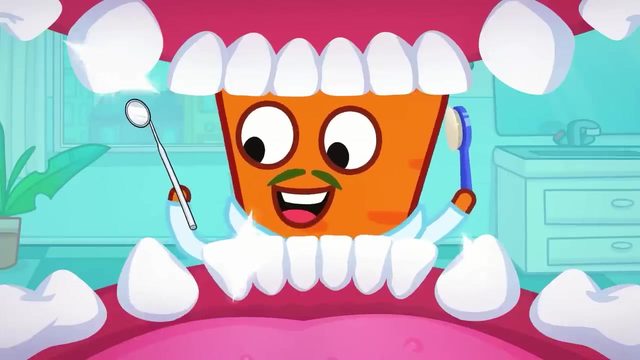 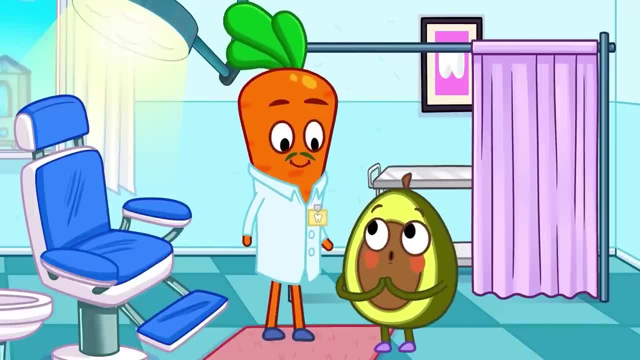 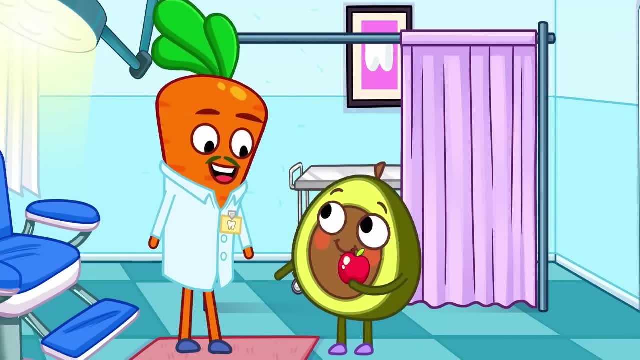 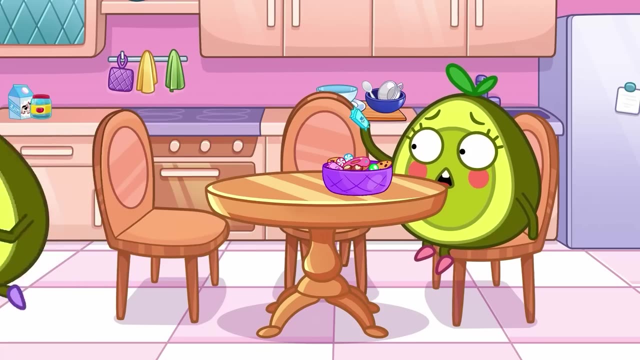 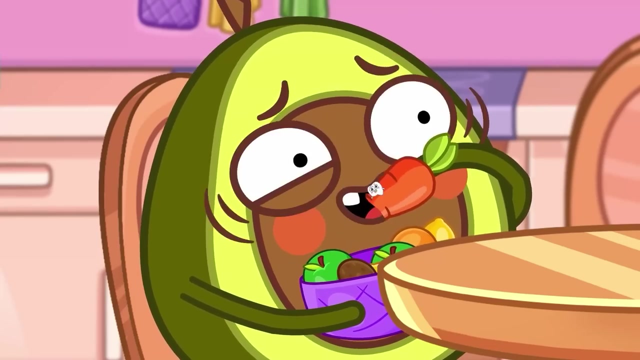 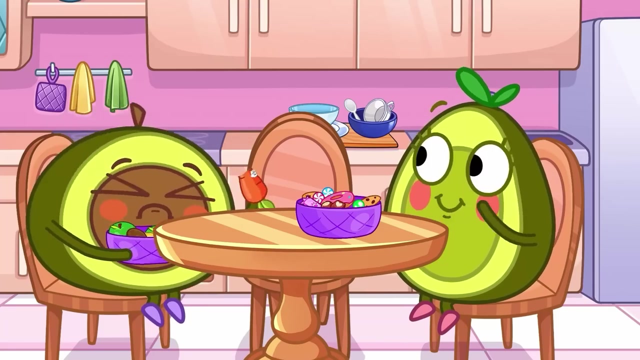 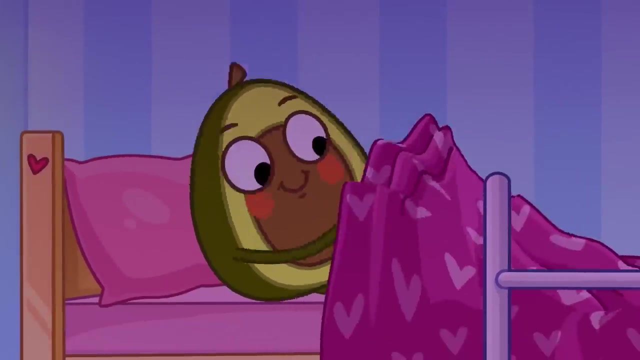 Visit the Tooth Fairy, Visit the dentist and don't forget to brush your teeth, Thank you, And eat healthy food. Do you want some candy Pit? What's that on your carrot Pit? Your baby tooth has fallen out. What did the Tooth Fairy bring? 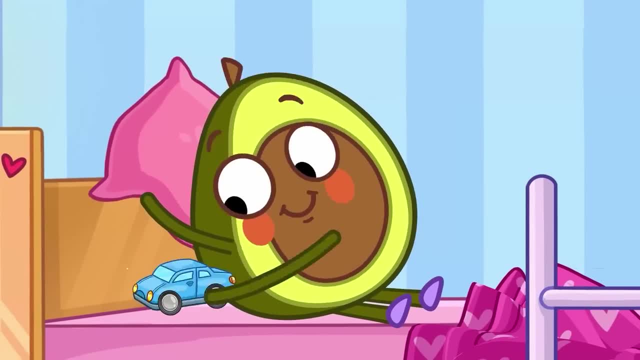 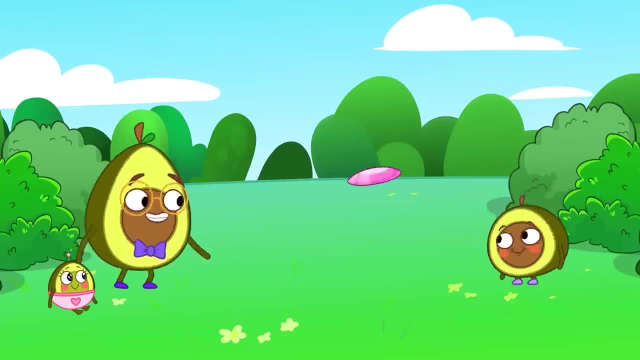 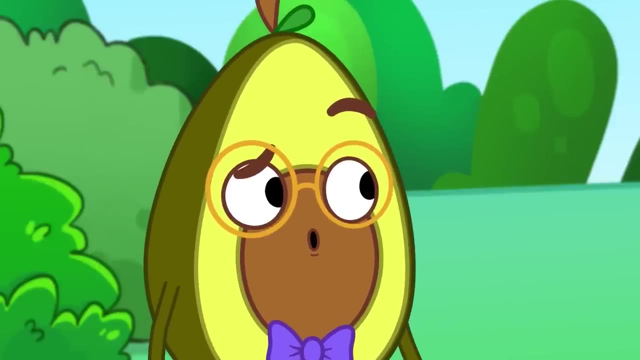 A toy car And new tooth is on the way. The family is playing frisbee And St injected him a lot of候. It helps people tobringy Inside, But where did Pit go? Brrr, GRRR. 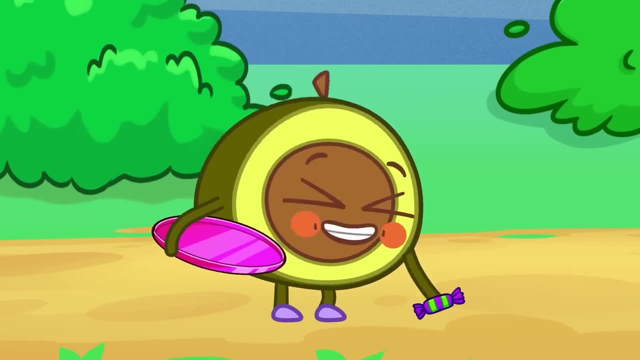 Let's say he's very hard too. WHop, And the happy hanging pot got ripped. Yay, He's found a trail of candy and one even has one WHOO Pit. You don't know who left them there. 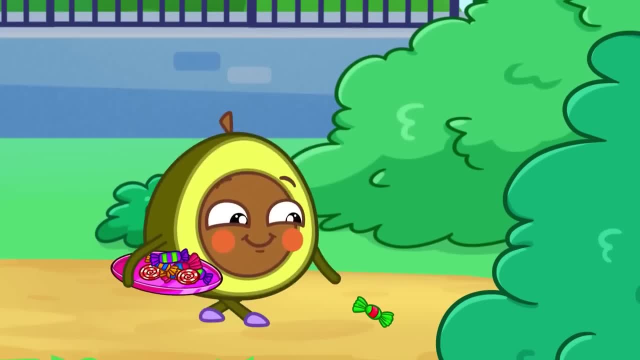 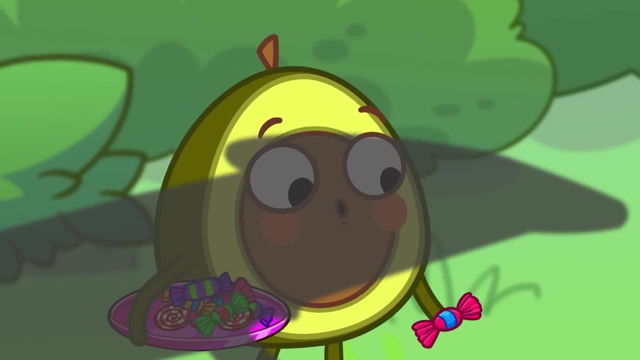 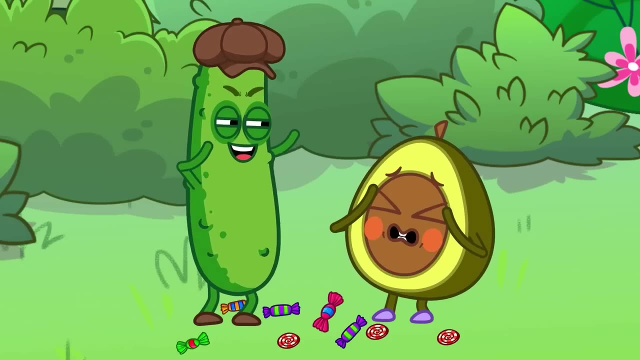 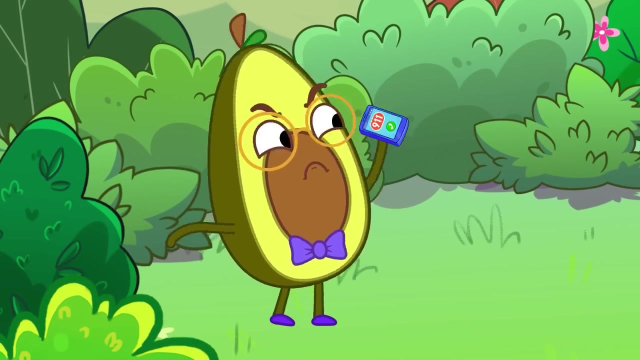 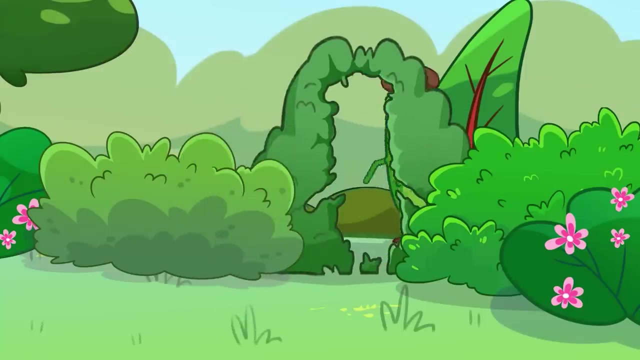 Stop it To. Through the rush of traffic Toигth through the대道. descriptions mean of our journey. Don't be pelaged on people who got stolen. What będą? Let's go Go fast. Good luck, Daddy. pit needs you get away from my son? daddy called 9-1-1 for help. never run away from your. 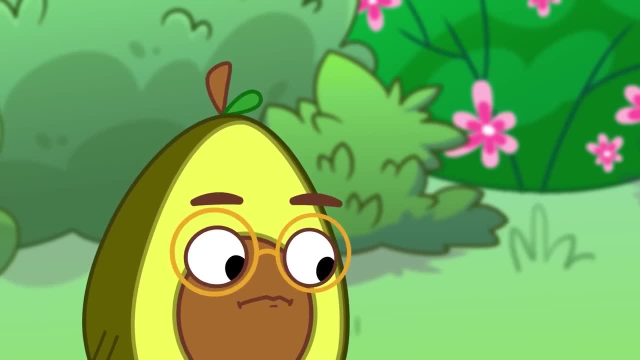 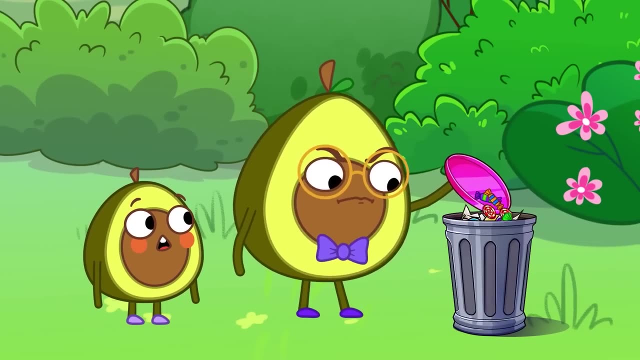 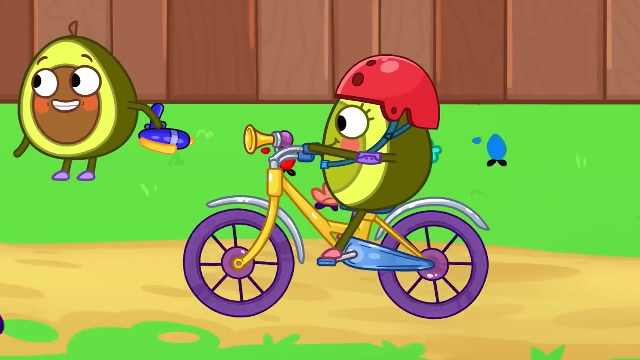 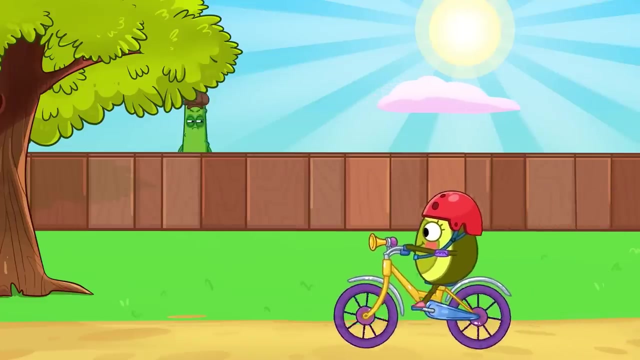 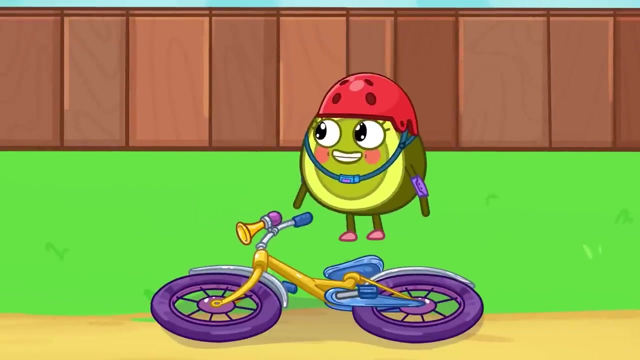 parents. don't let strangers touch you. you need to throw all that candy away and don't take anything from strangers. penny is riding her bike while pit plays with his squirt gun. oh no, that stranger is back. he's offering penny some ice cream. don't take it, penny. 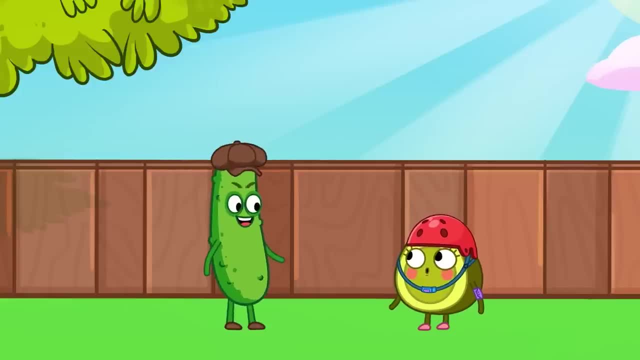 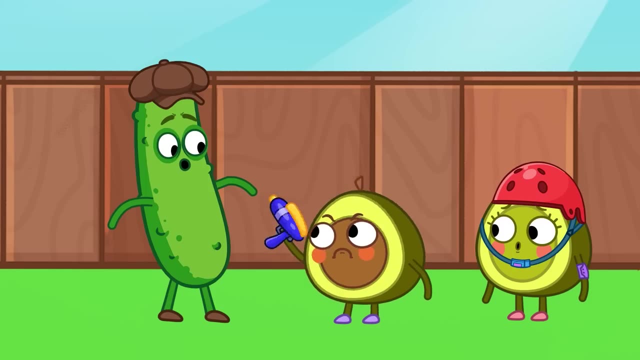 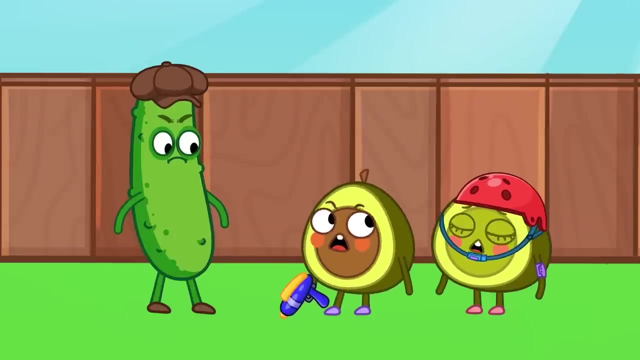 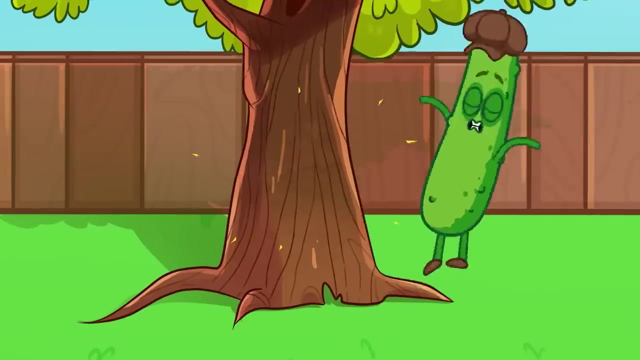 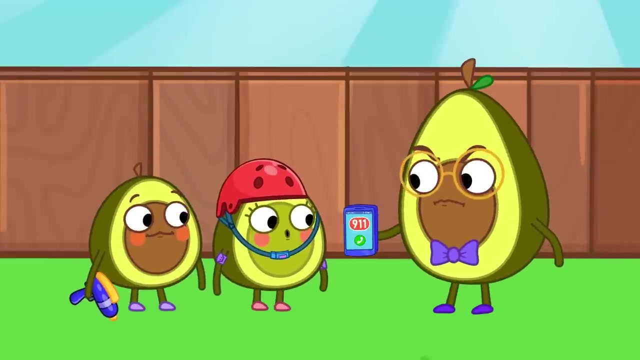 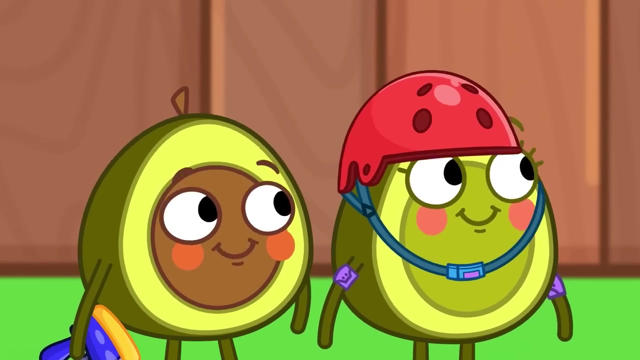 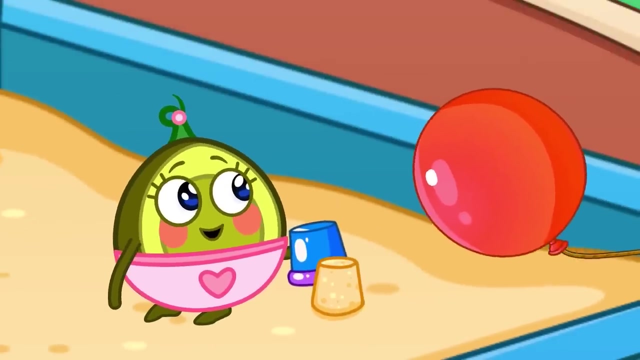 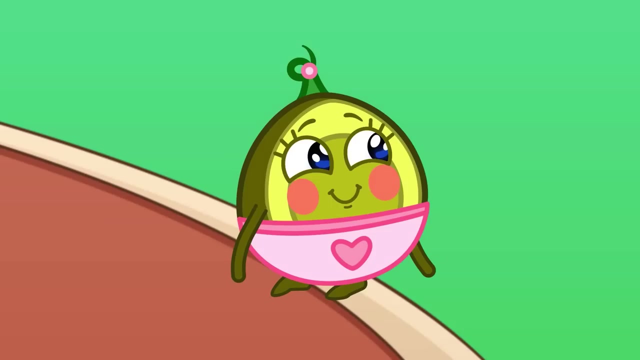 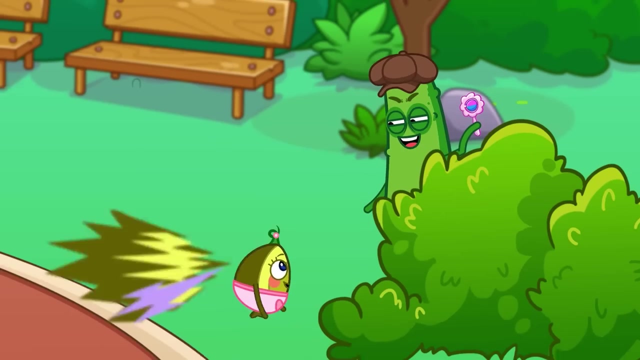 come quick. the stranger is getting away again. what should they do if you're not here, if your parents aren't around, call 911. baby loves balloons. the stranger is using it to trick baby. oh baby, baby, baby. Baby needs your help. Penny, do you remember what to do? 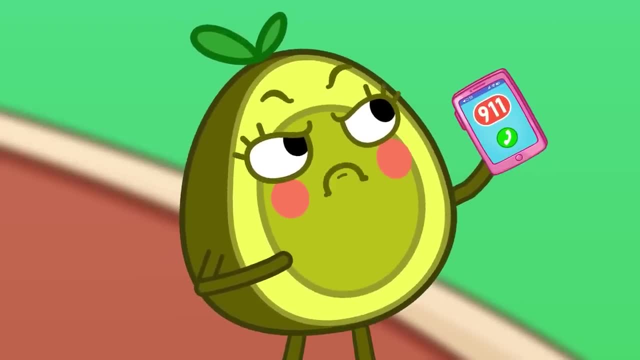 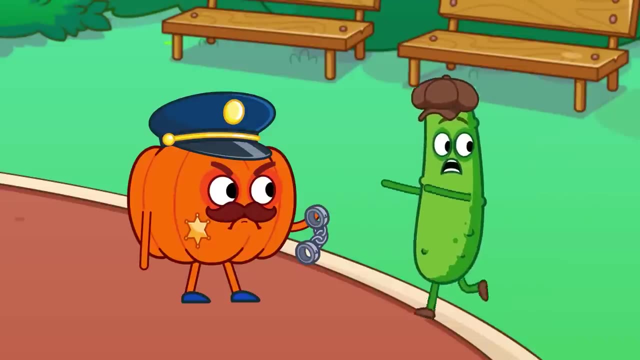 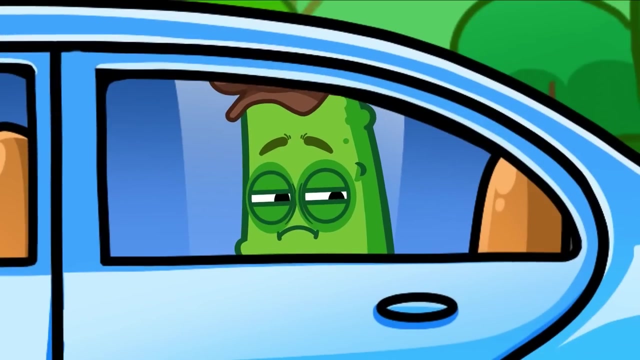 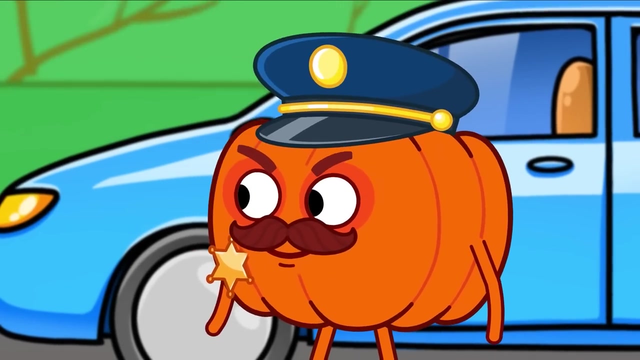 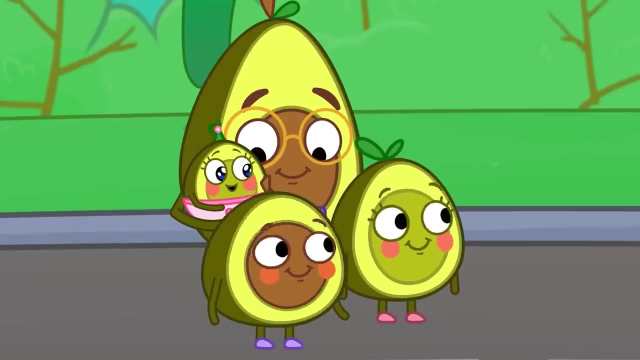 Go away, stranger. I'm calling 911!. Phew, Daddy's here, And so is Officer Pumpkin. Don't let strangers touch you. Always call your parents and dial 911!. Don't worry, Officer, They won't forget. 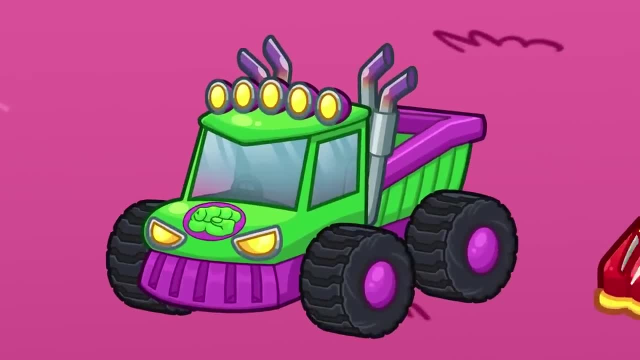 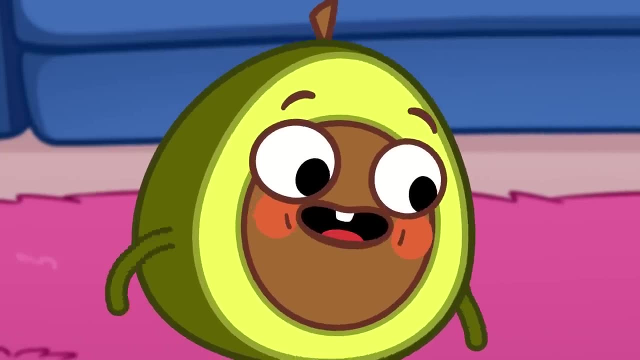 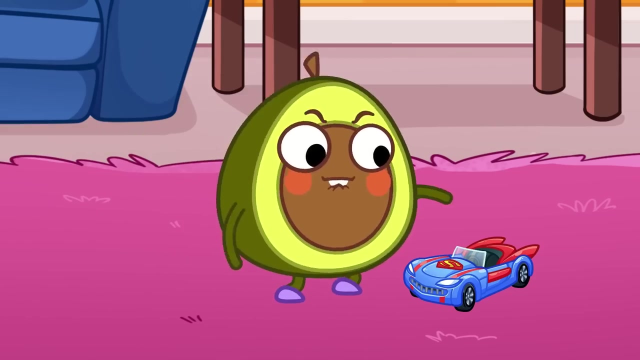 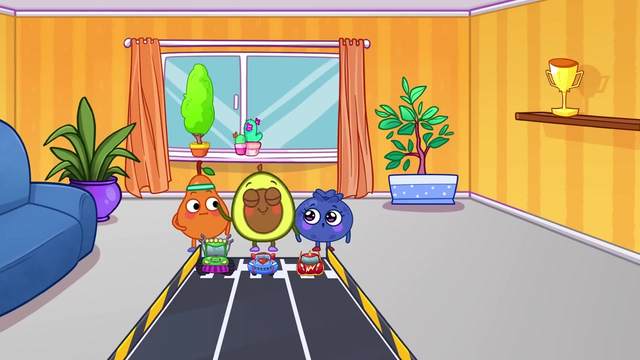 Ooh, Free toy cars: Smash'em Truck, Flashmobile and Super Racer. Pear wants Smash'em Truck, Blueberry wants Flashmobile. That leaves Super Racer for Pits. Let's have a race And the winner gets a trophy. 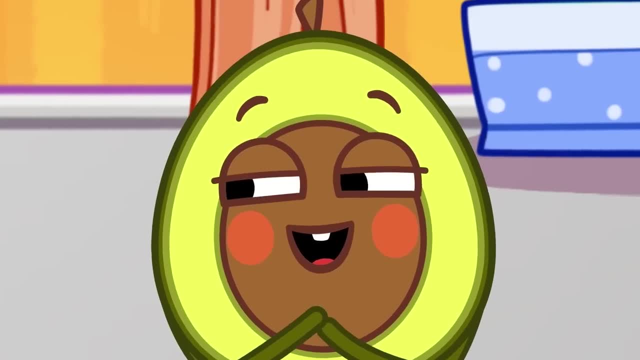 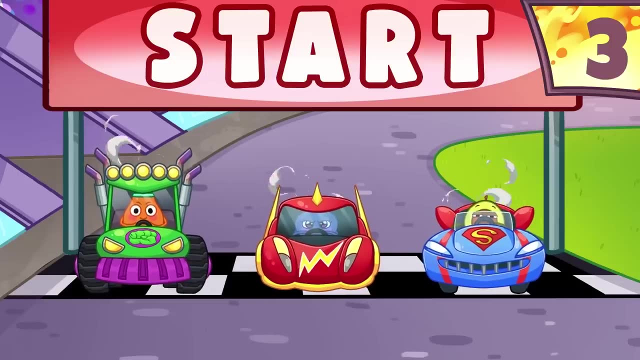 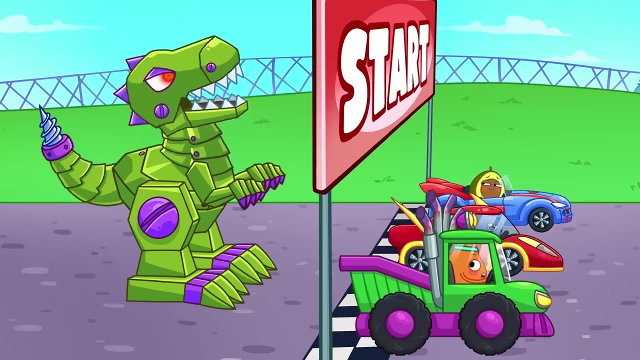 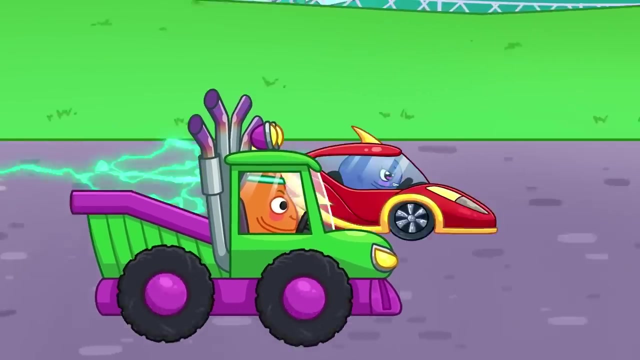 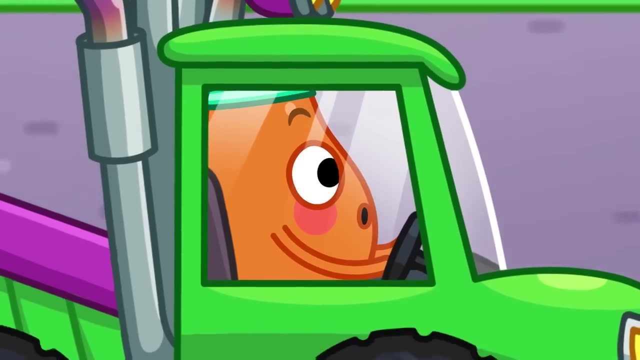 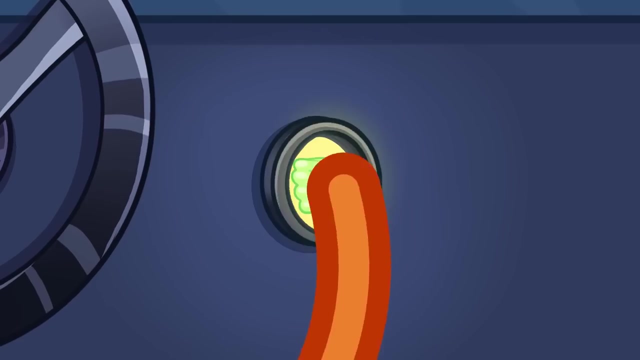 But watch out for the T-Rex On your mark… Get set… Go. Blueberry takes the lead And there goes Pit, See ya, Watch out for the wall. This is a job for Smash'em Truck Hooray. 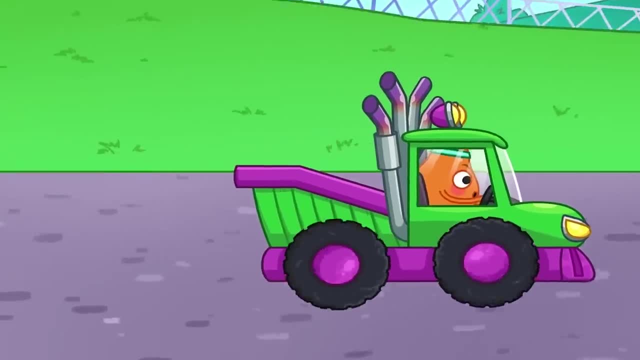 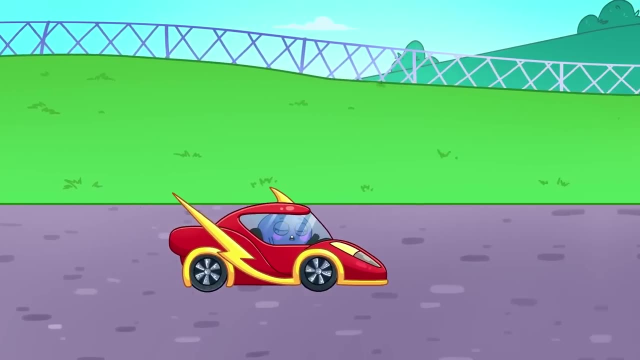 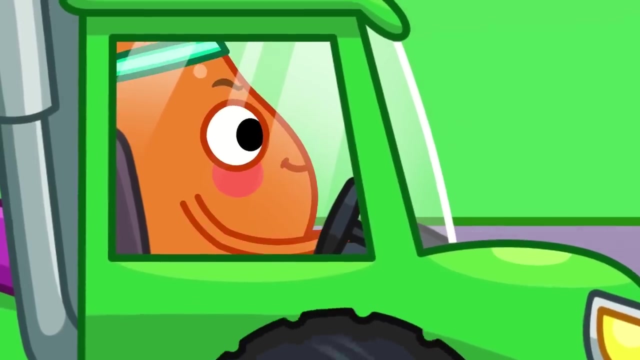 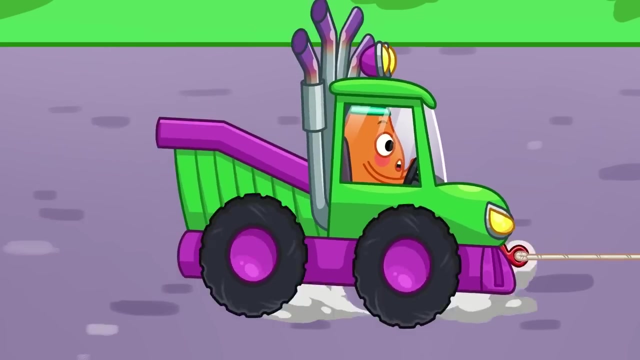 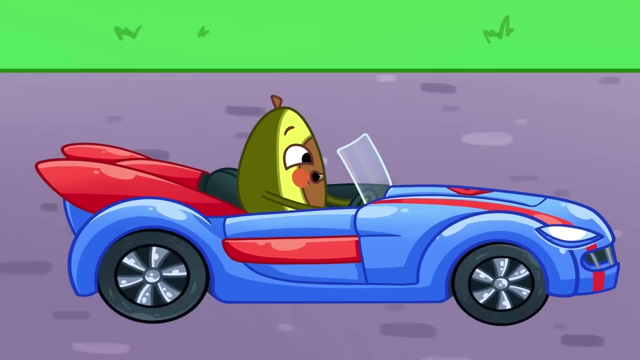 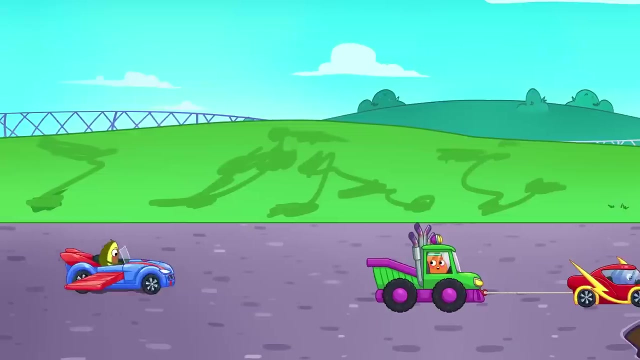 Hurry, It's the T-Rex Blueberry. can you help Pear Flashmobile to the rescue. Pull the trigger Pits. Oh no, That ditch is too wide And T-Rex is coming. Pit, can you help? 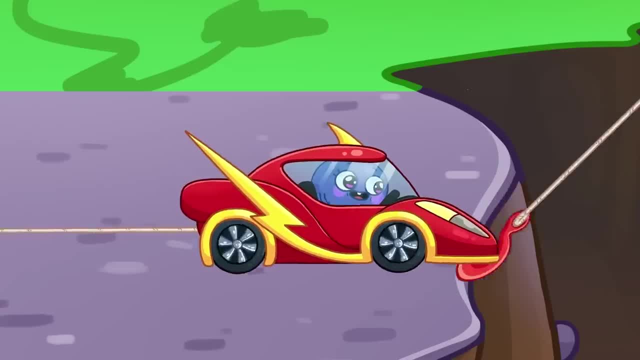 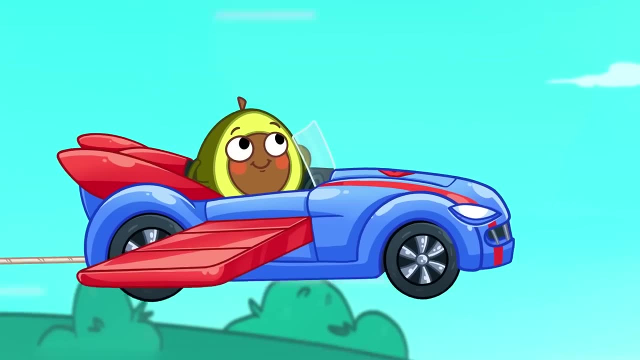 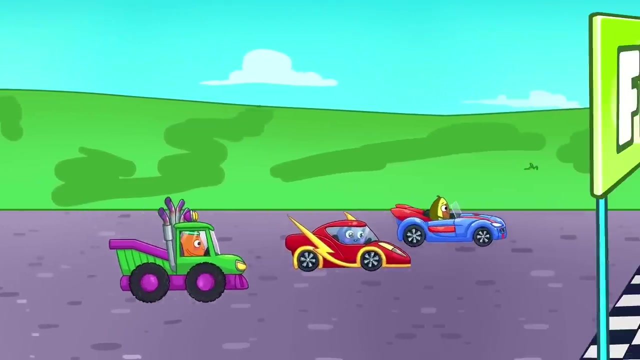 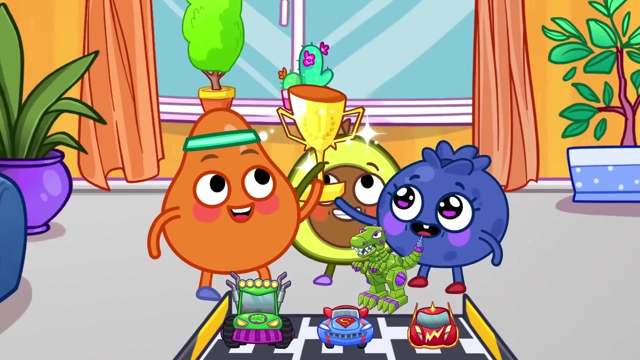 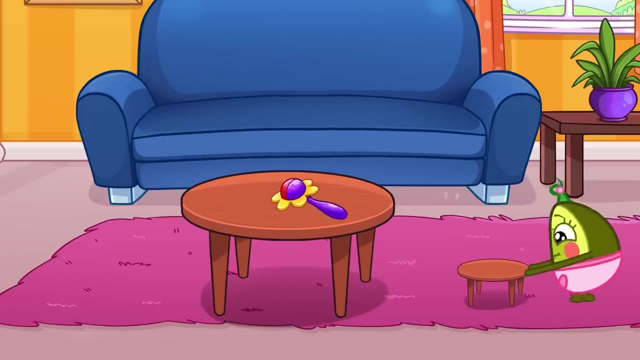 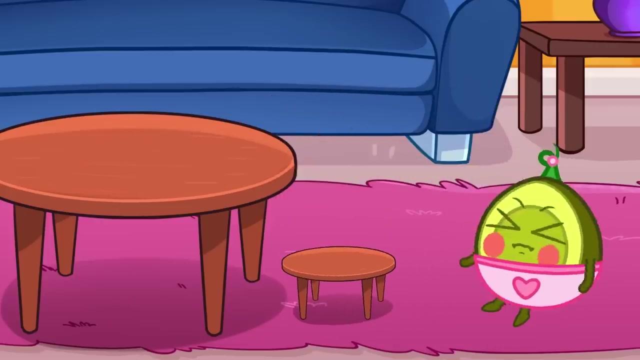 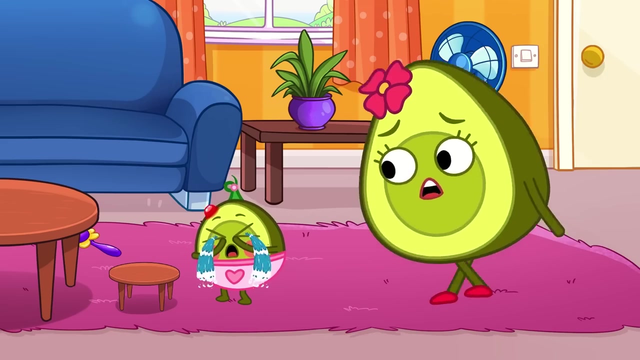 Well done, Pit. It's a tie, That means everyone's a winner. Baby wants her rattle, But be careful, Baby. Baby got a boo-boo on her head. Time for Mommy's boo-boo song. Baby, baby, dry your tears. 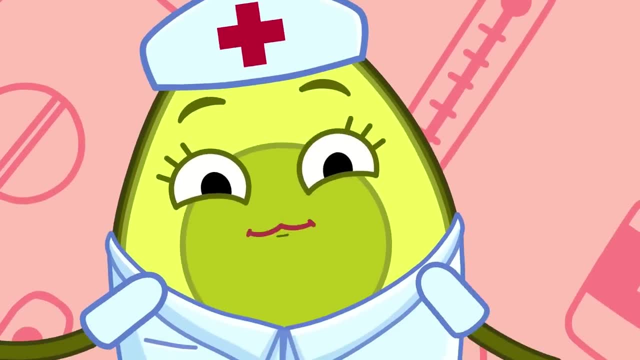 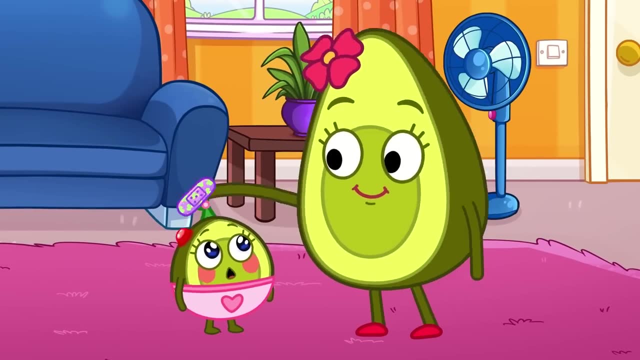 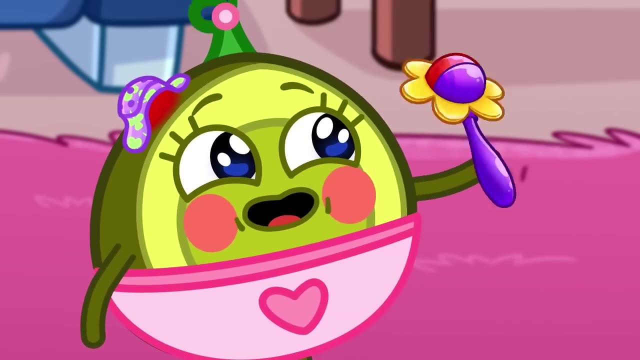 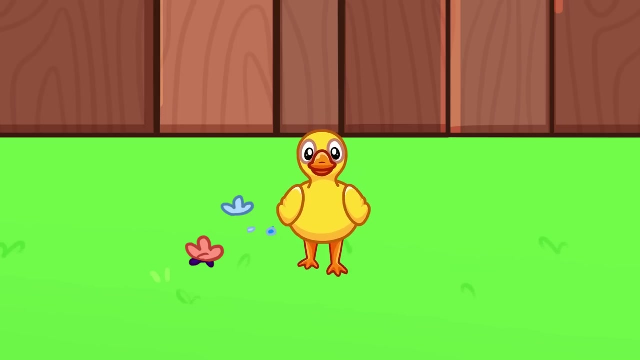 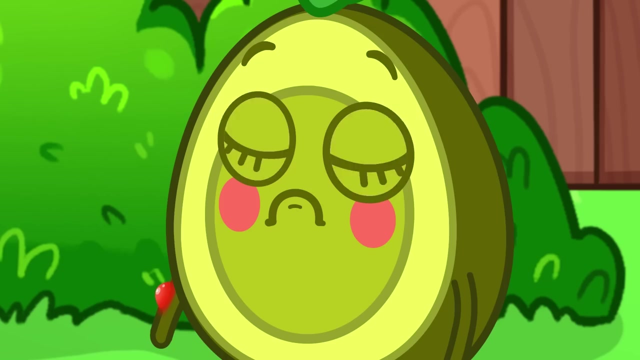 Fix your boo-boo, have no fear. Then they chant: Mommy peace. Fix your boo-boo now. Yay, Baby feels much better. Penny is riding her bike. Oh no, Watch out for the duck. Penny has a boo-boo on her arm. 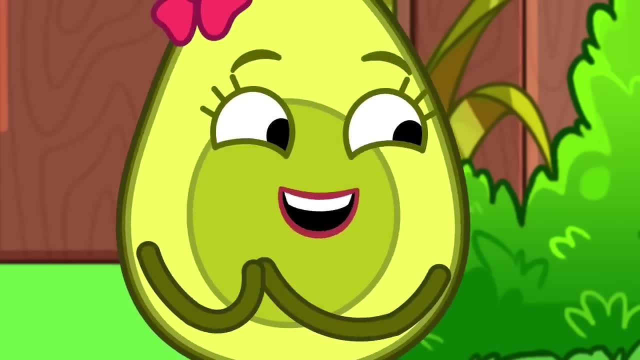 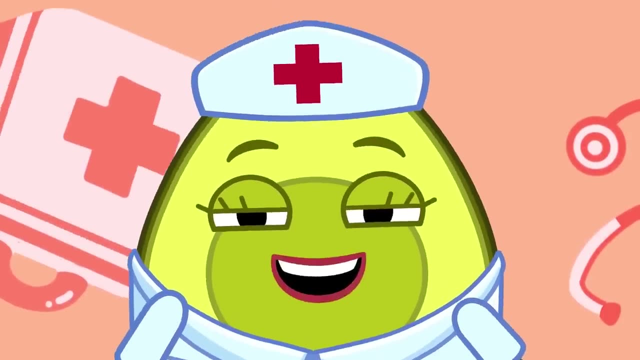 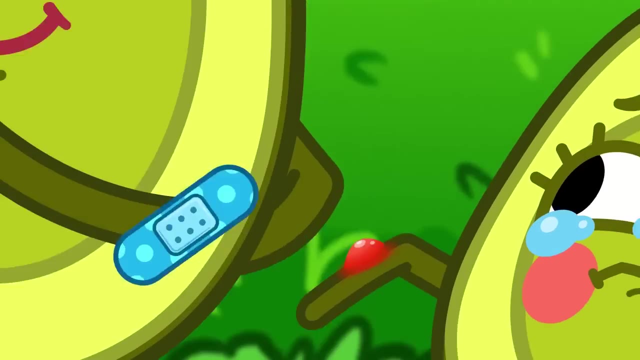 Hurry, Mommy, Sing your song. Baby, baby, dry your tears. Fix your boo-boo, have no fear. Then they chant: Mommy, peace. Fix your boo-boo now. Penny is ready to ride her bike. 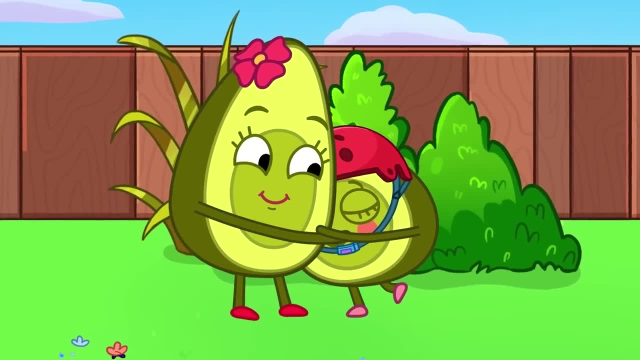 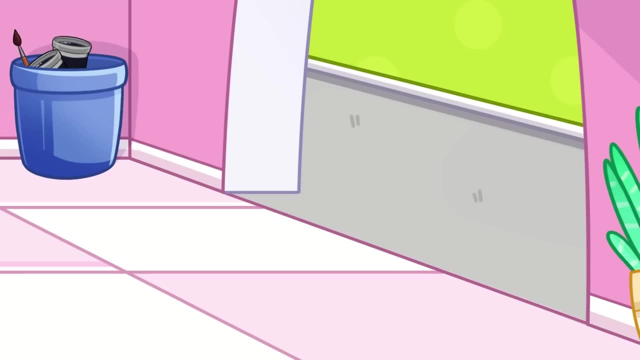 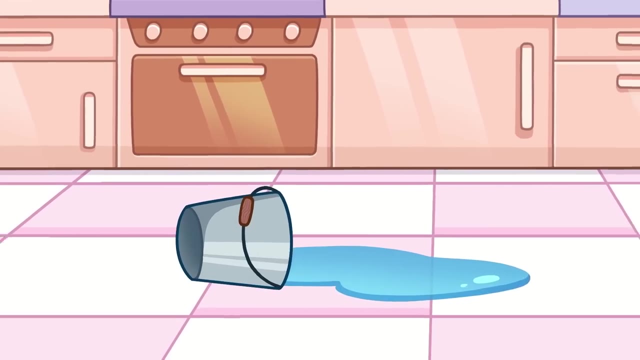 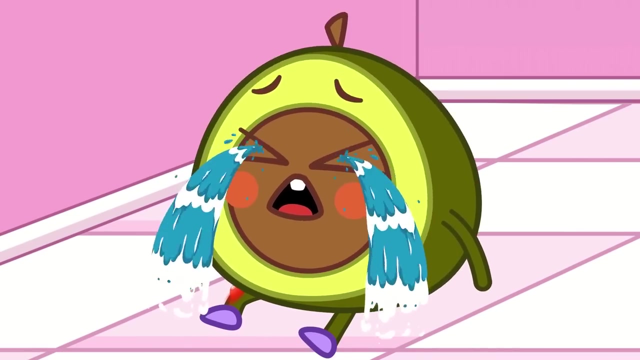 But don't forget your helmet. Pit is playing with his toy car. He-he-he, Oops, Now there's water on the floor. Pit has a boo-boo on his knee. We need Mommy's boo-boo song. Baby, baby, dry your tears. 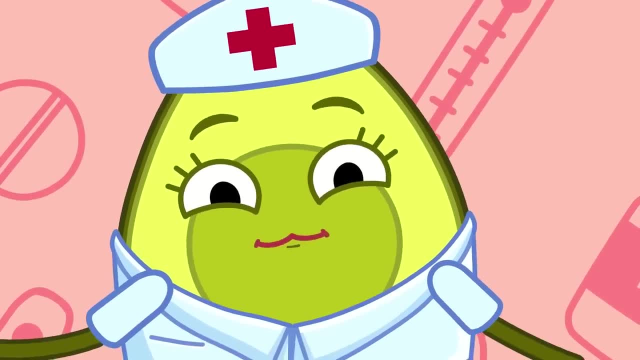 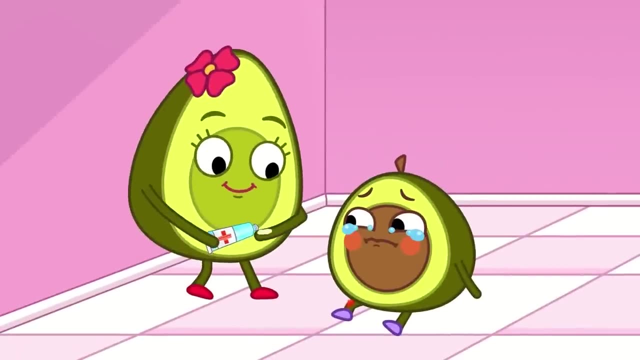 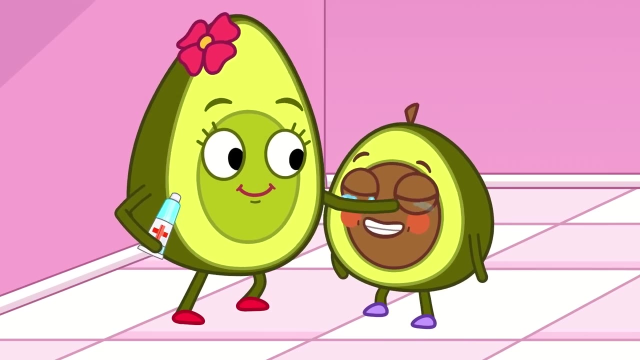 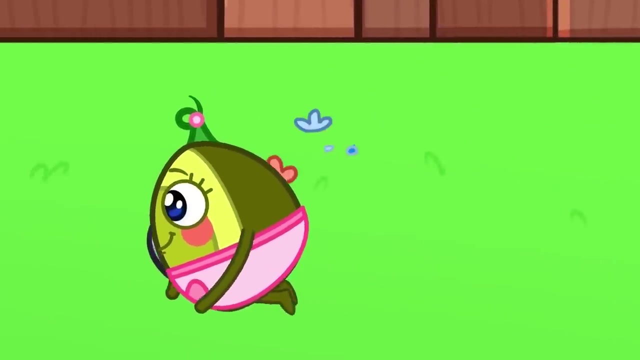 Fix your boo-boo, have no fear. Then they chant: Mommy peace, Fix your boo-boo. now. Mommy puts ointment on Pit's boo-boo. Hmm, It's all better now. Baby is being careful. 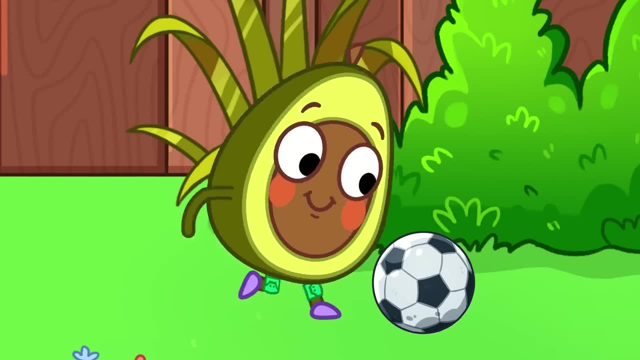 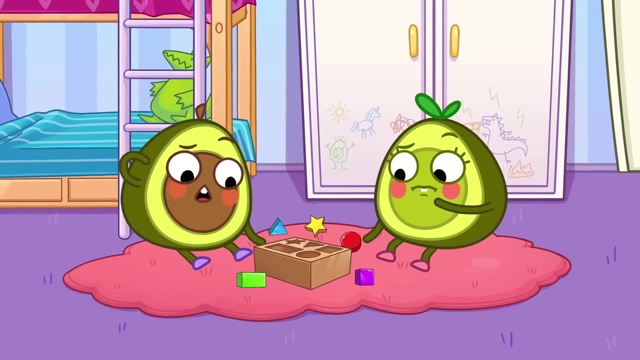 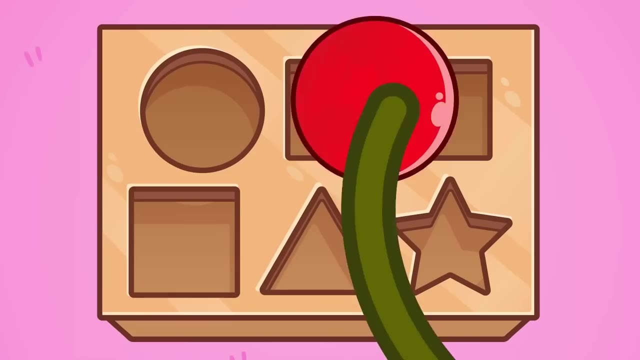 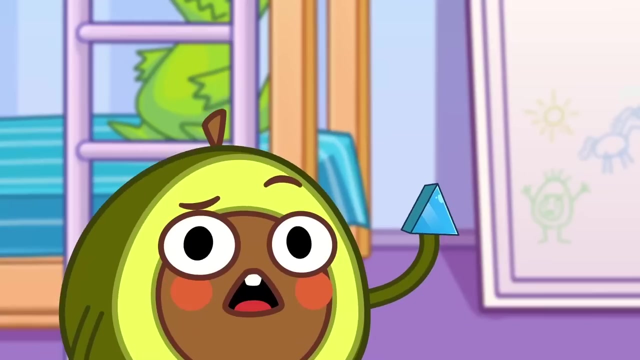 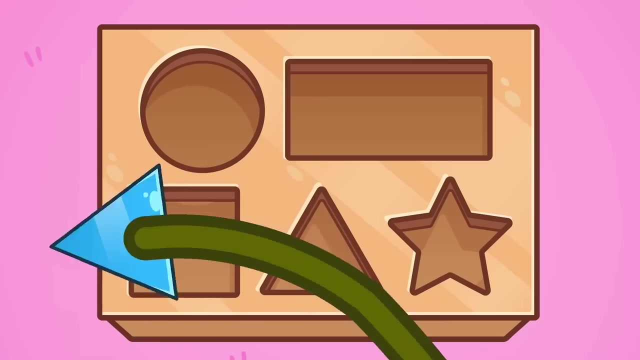 Penny is being careful And Pit is being careful too. This all makes Mommy very happy. Pit and Penny need to match the right shape with the right hole. Good job, Penny. Yeah, Yeah. Now Pit needs to find where the triangle fits. 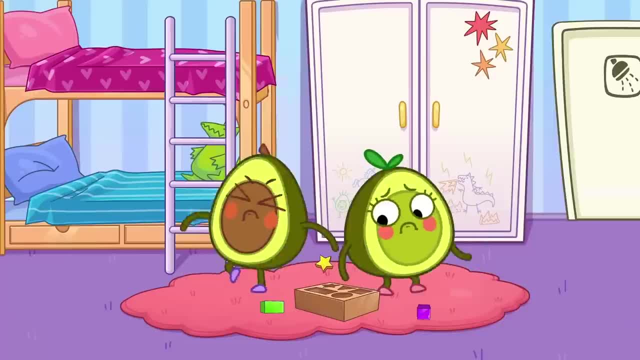 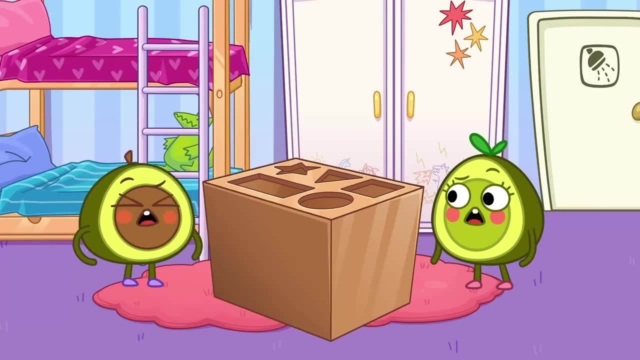 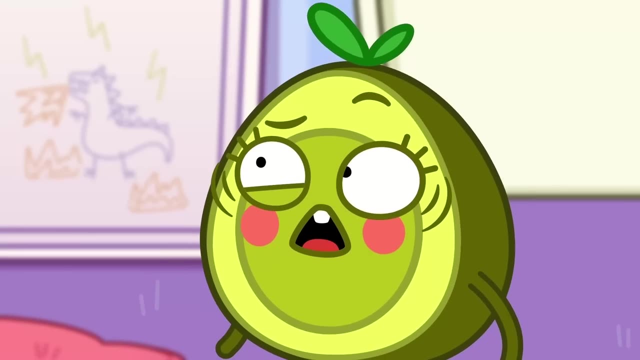 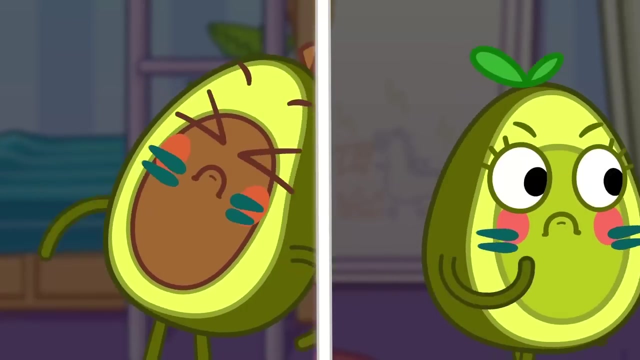 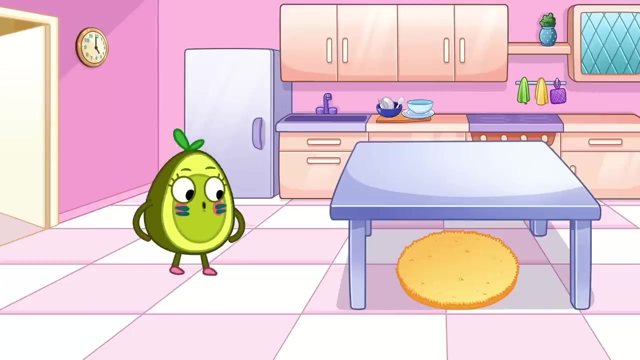 Pit doesn't want to play anymore…. Hmmm, What does that mean? Pit needs to try and change his role as well. Hehehe, The shapes have come to life. Oh no, The shapes have run away. What shape is the rug Penny? 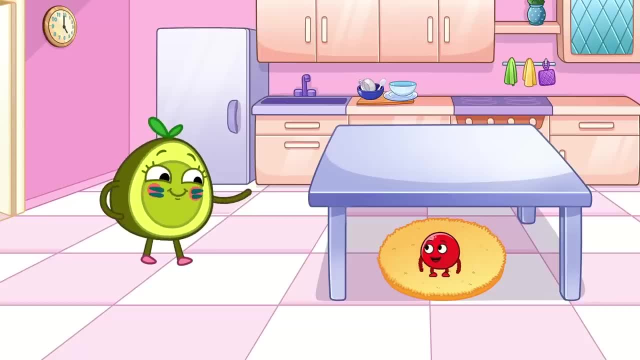 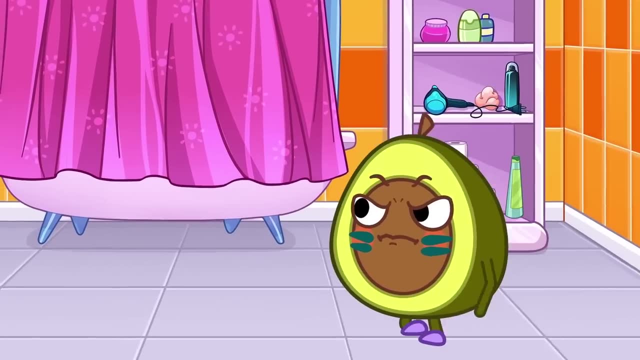 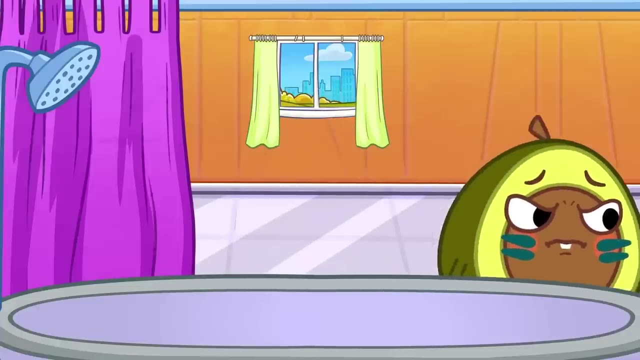 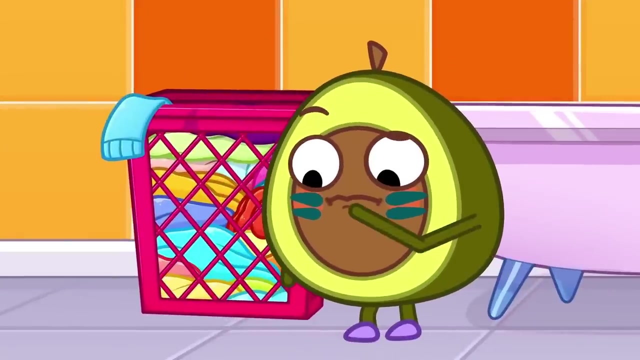 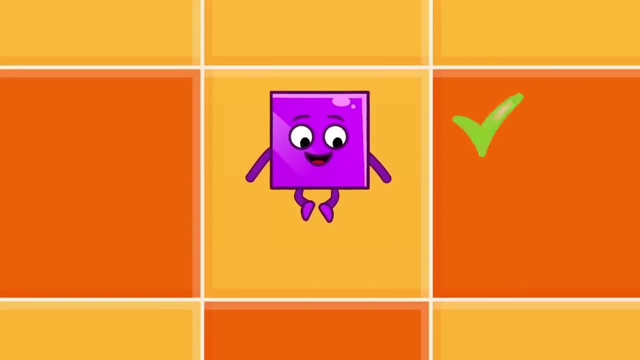 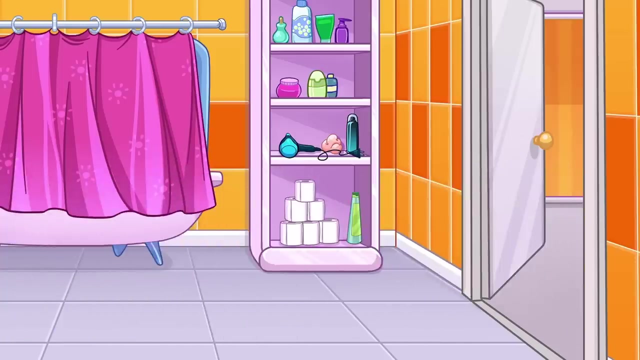 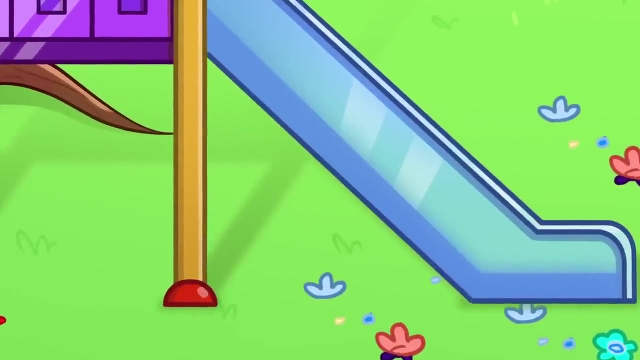 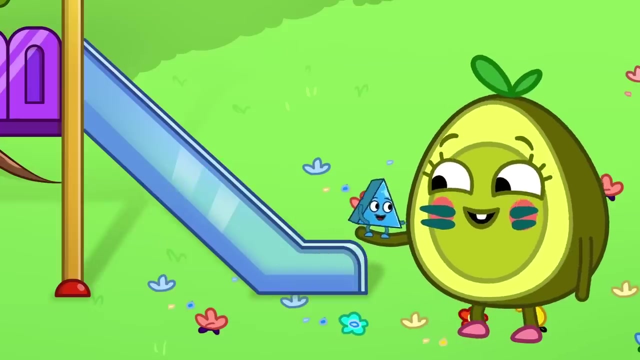 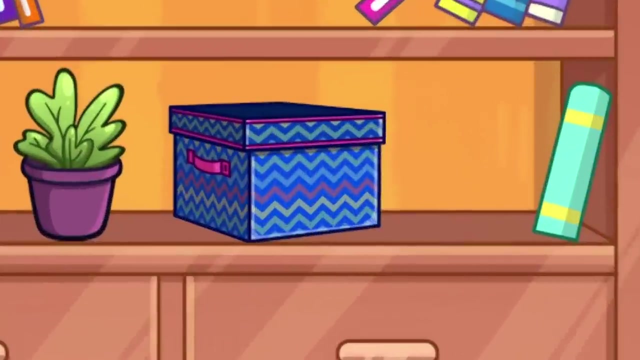 Yay, You found Circle. What shape is the tile? Pit Square Square? It's Square. That's right, it's square. What shape is this Triangle? It is, it's triangle. Do you know what shape this is? 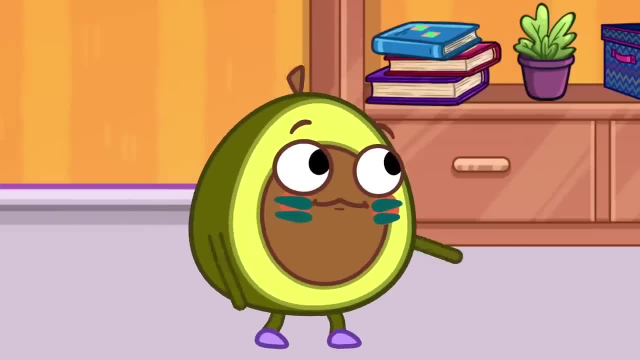 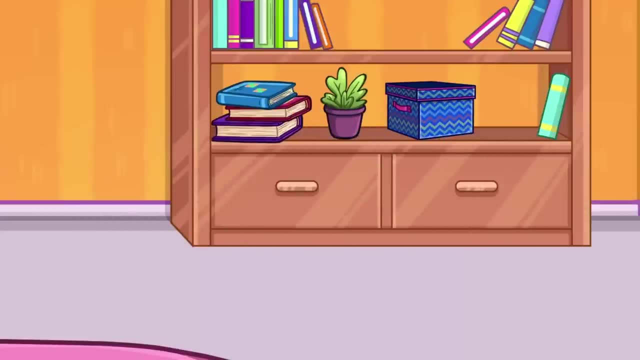 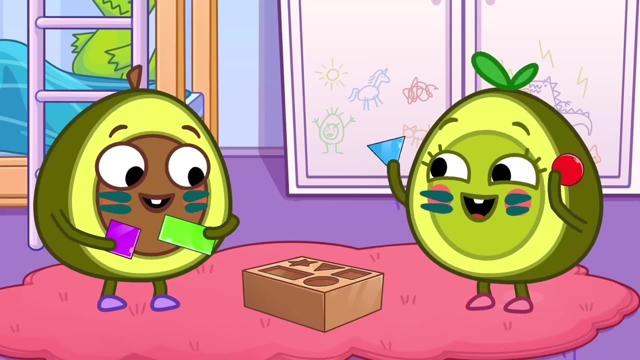 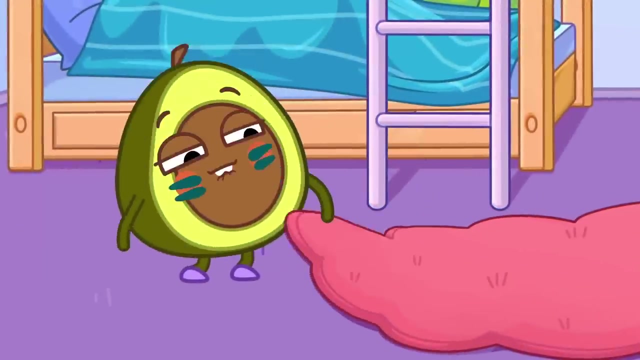 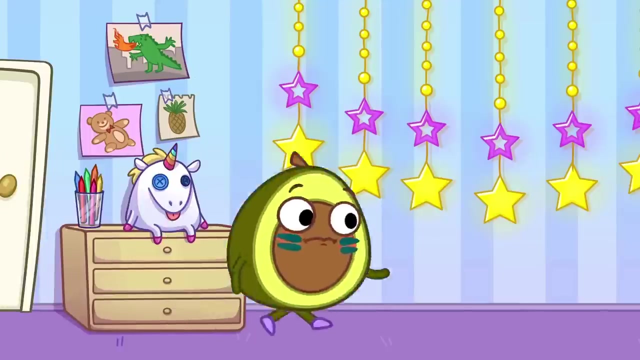 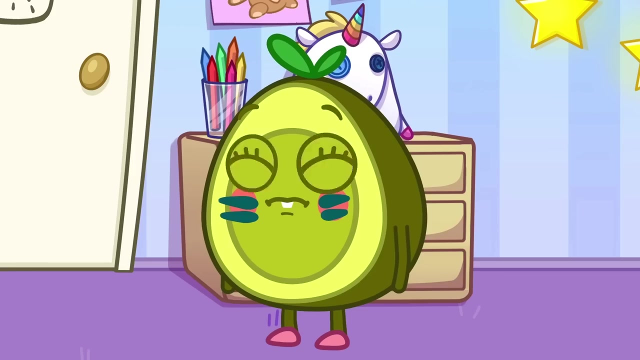 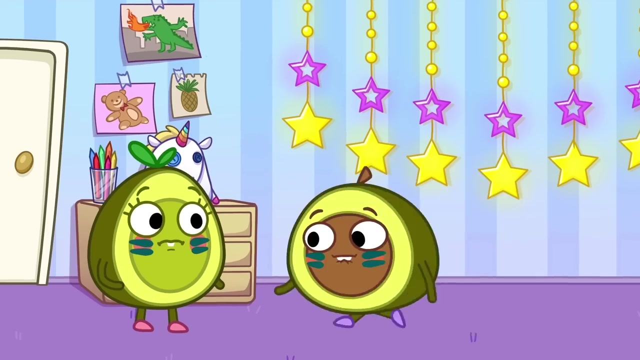 Do you know this shape? Pit Rectangle. Correct, It's Rectangle. Now you can put the shapes back where they belong. But where's Star Under the rug, Behind the curtain Rectangle? Do you see Star, Penny Star. 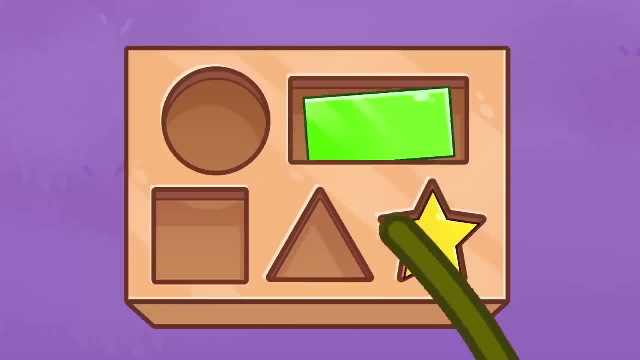 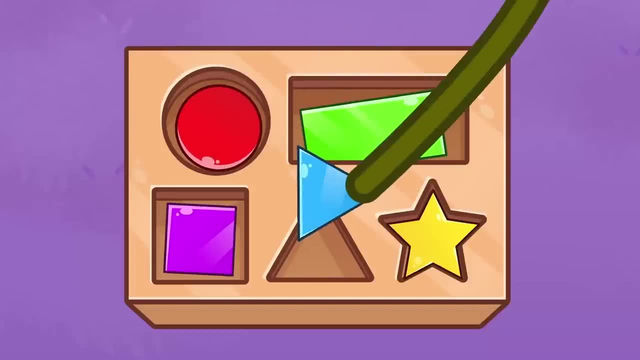 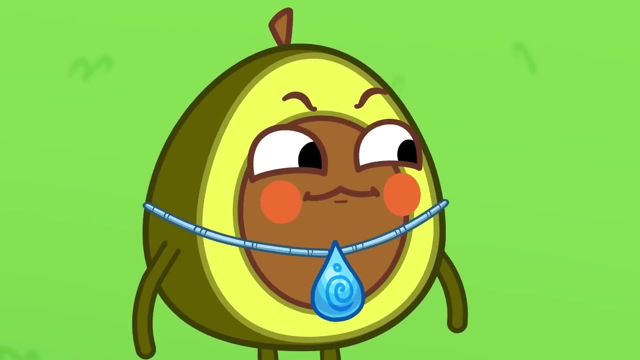 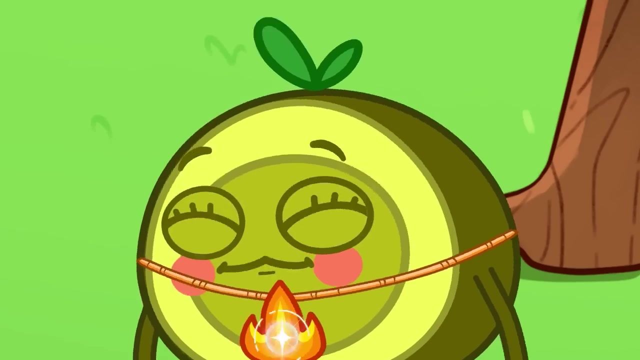 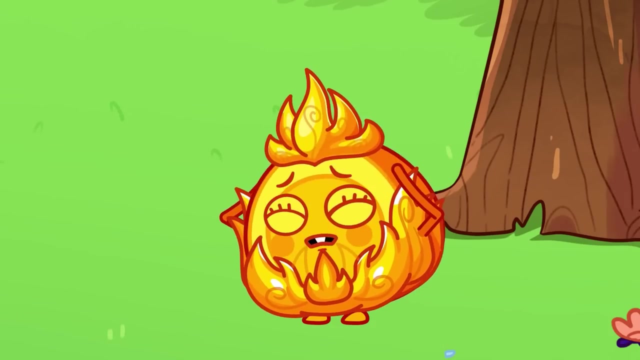 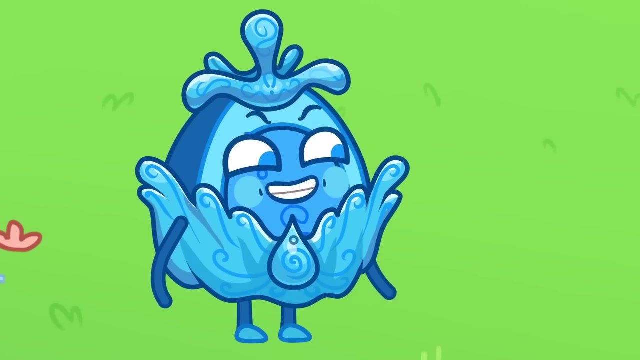 Let's see if the kids know their shapes: Rectangle, Square, Circle And triangle. Well done. Pit has a magical necklace And Penny has one too. Pit can control water, Oh, And Penny can control fire. Water can put out fire. 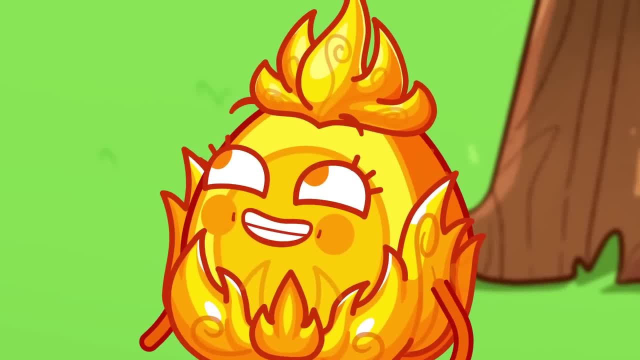 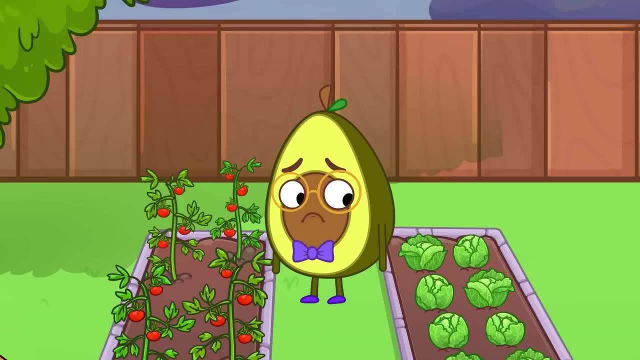 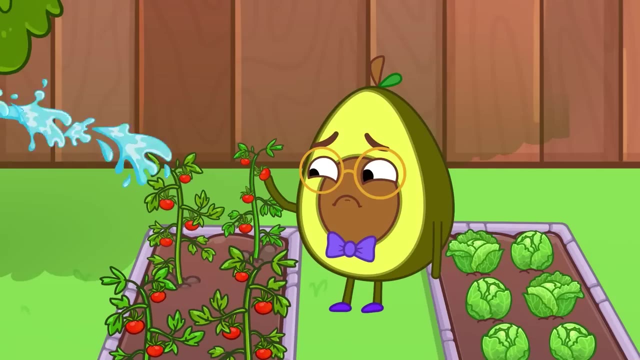 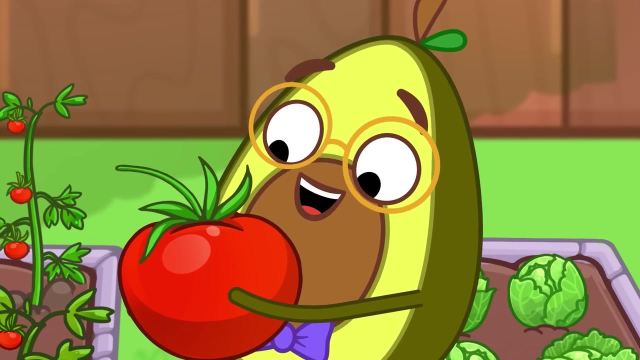 Can you do that, Penny, And you can destroy all of it. Your plan is complete. Hehe, KISH, Daddy's vegetables don't look very good. Maybe Pit can help. Water helps plants grow, Haha, Duh. 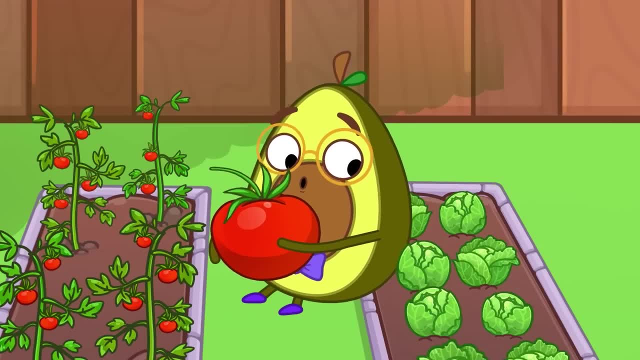 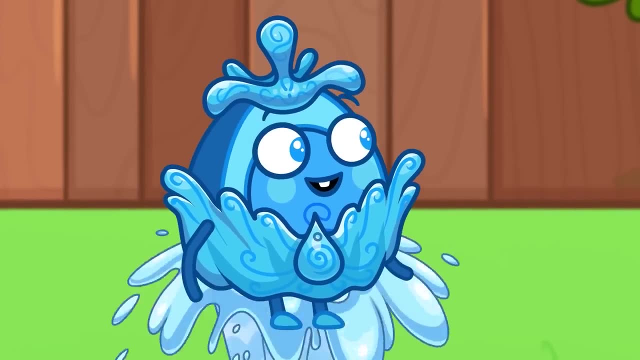 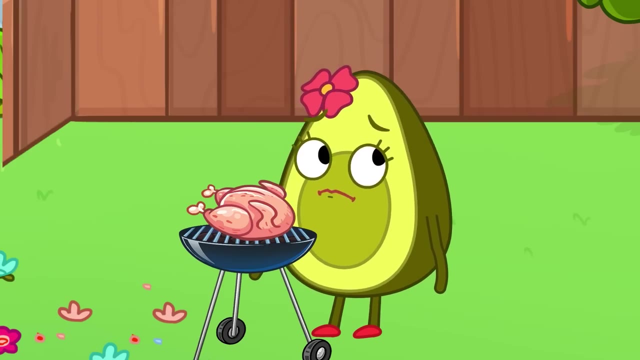 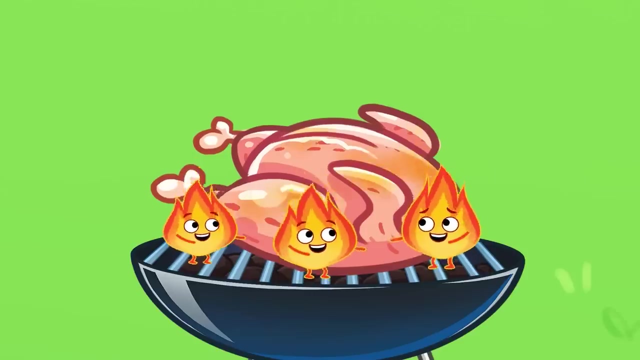 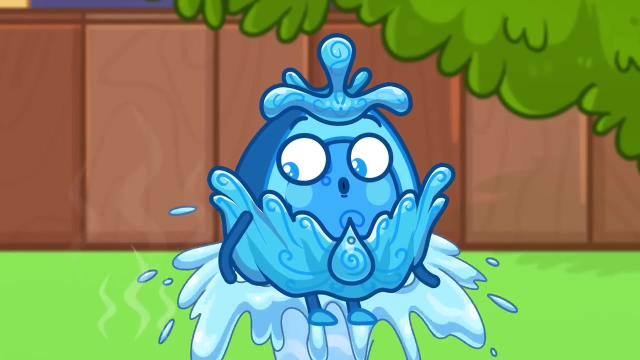 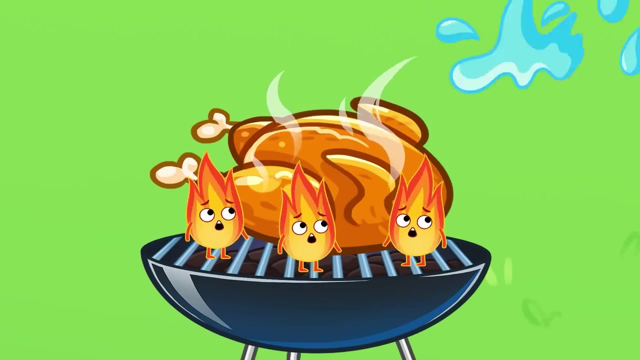 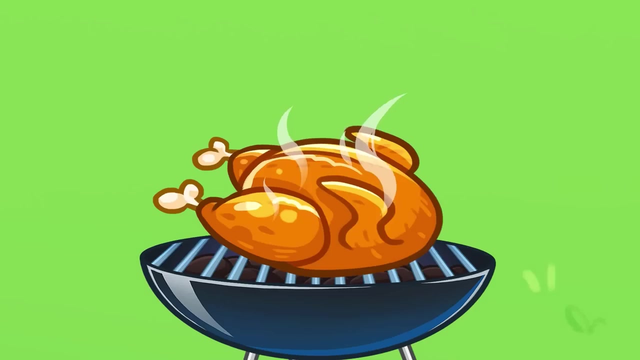 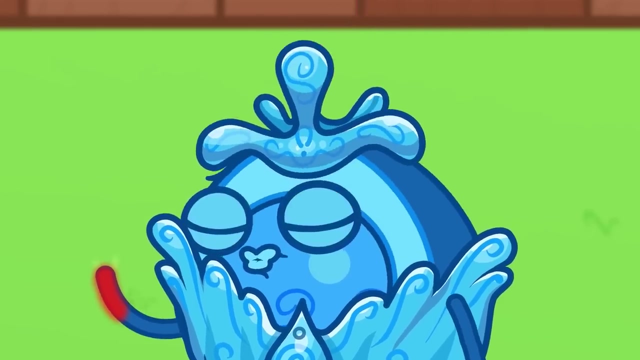 Ah, Haha, Oh, Mommy needs help cooking. the chicken Fire helps things cook. Now Pit wants to eat some chicken. Yum, Uh-oh, what is Penny doing? Be careful, Pit. Oh no, The fire is out of control. 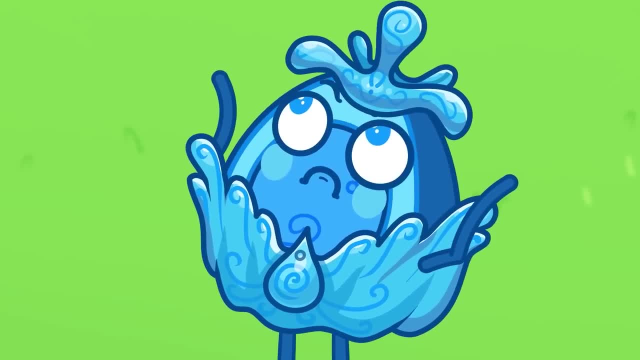 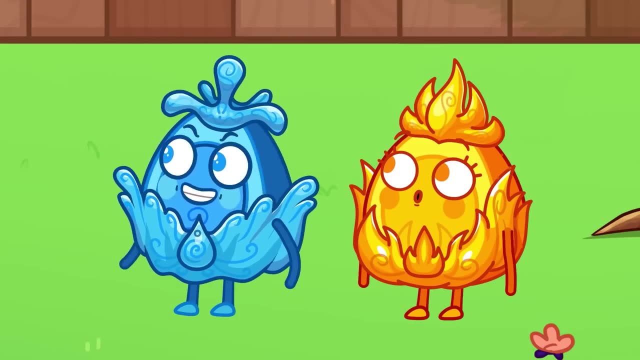 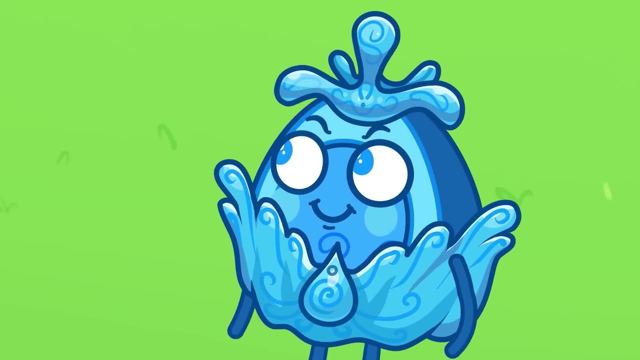 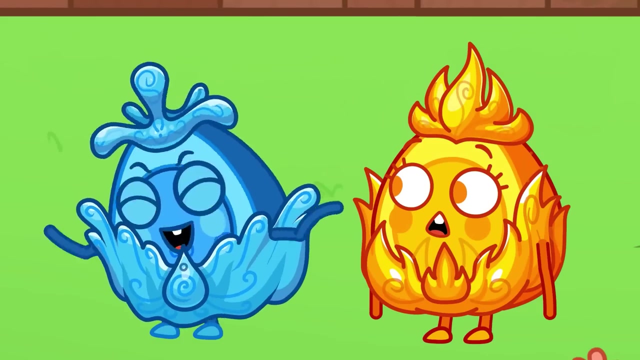 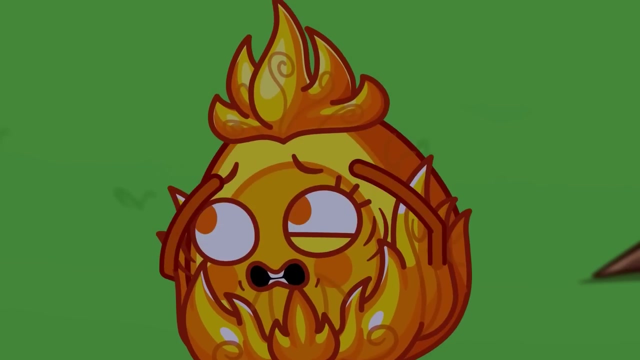 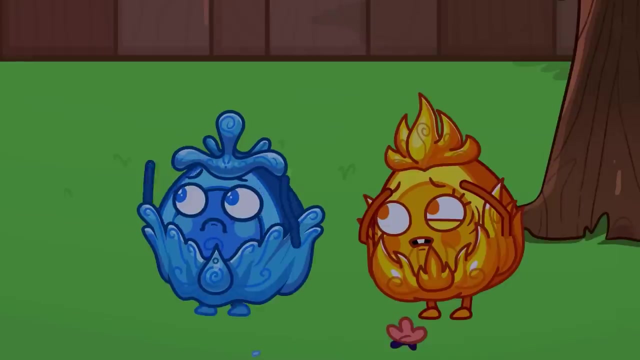 It's too strong now. Maybe a rain cloud will help. It's working. More, More Now. the cloud is working. Now the cloud is working. Now the cloud is a tornado. Oh no, What have I done? Stop Pit. 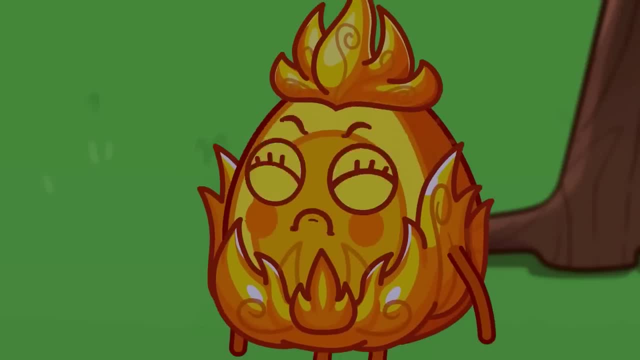 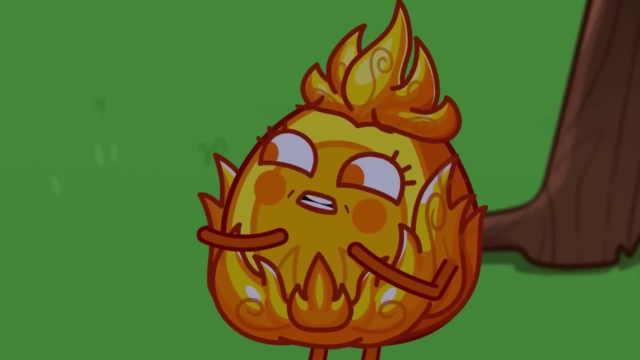 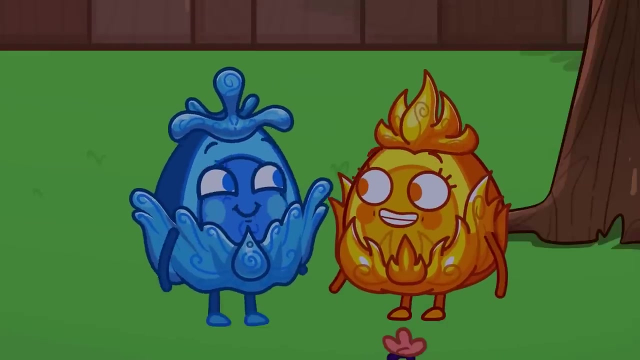 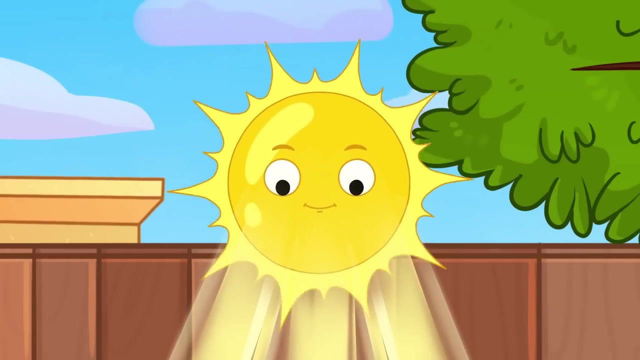 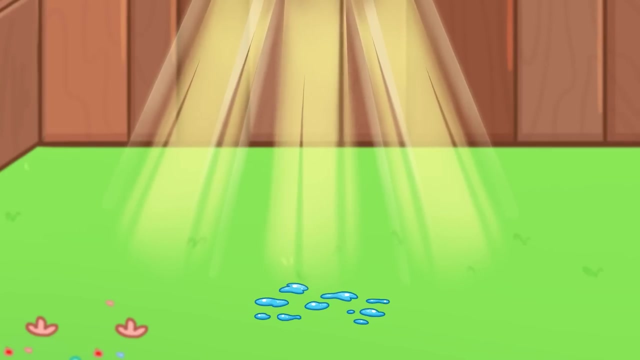 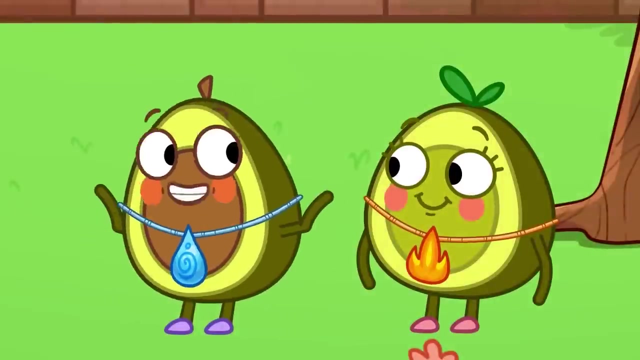 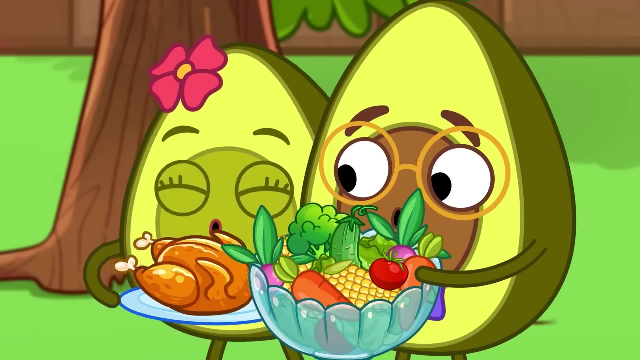 That made it bigger. Maybe Penny can help. What should we do? Pit has an idea. The sun will chase those clouds away And make the tornado disappear. Pit and Penny did it. That's why fire and water should be friends. Fire and water helped make lunch. 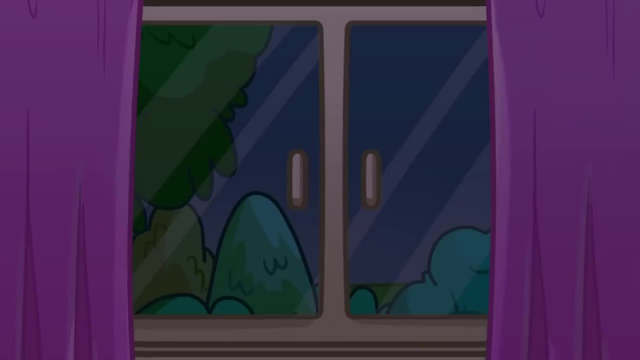 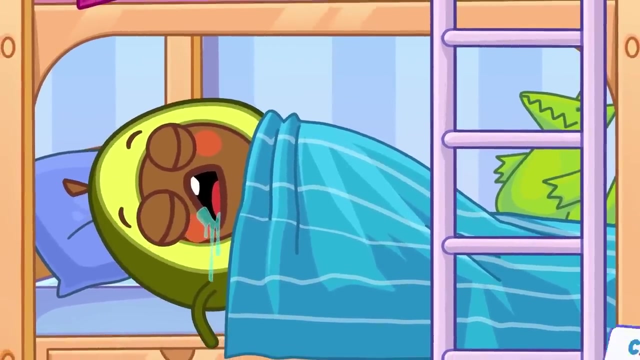 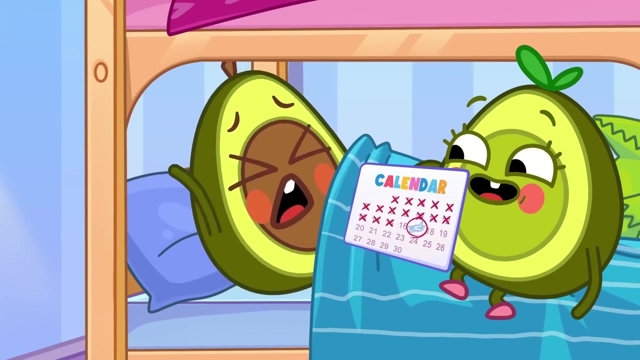 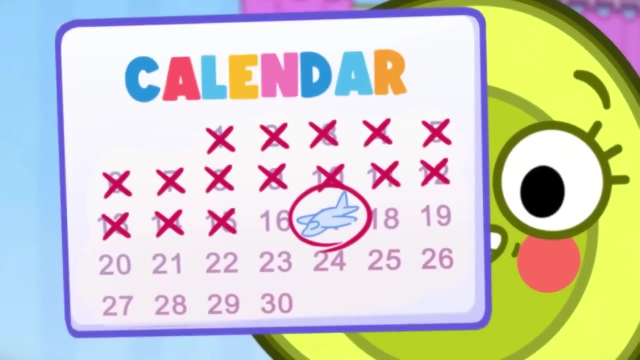 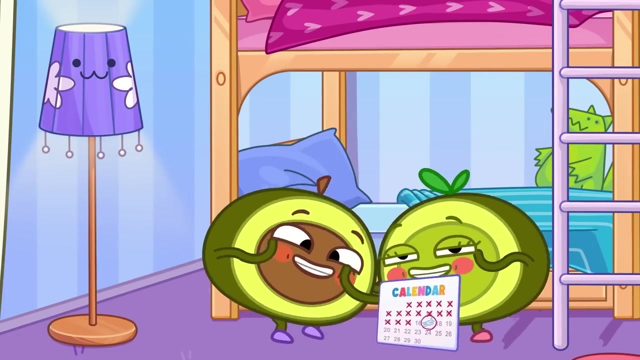 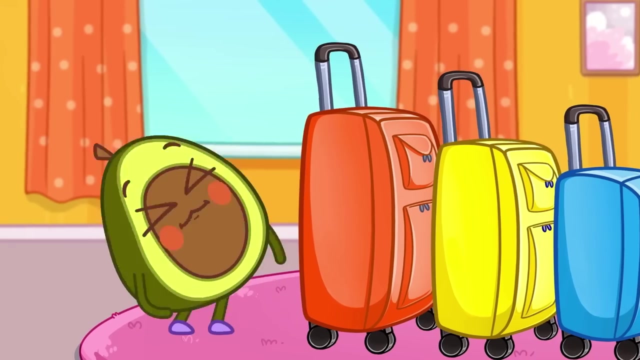 Well done, Pit and Penny. Shh, Pit is sleeping, But Penny has something to show him. What is it, Penny? They're going on a trip tomorrow. Hello, Exciting. The suitcases are already packed. Be careful, Pit. 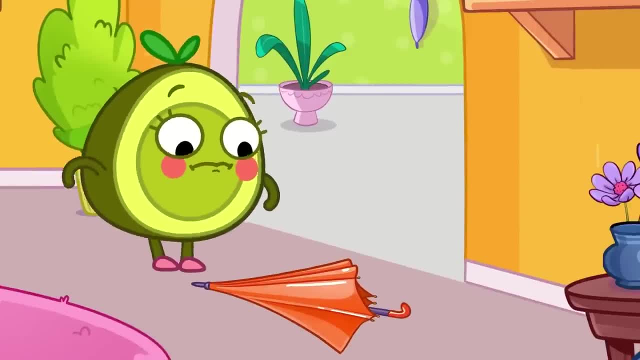 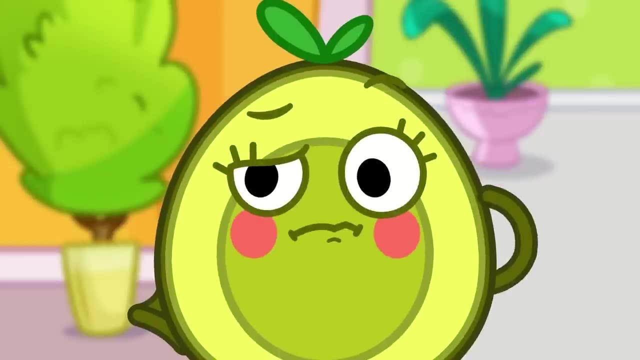 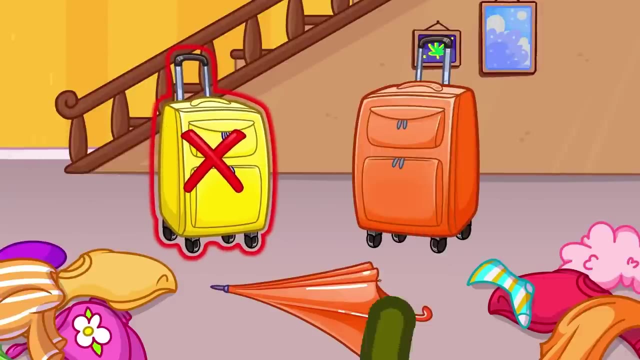 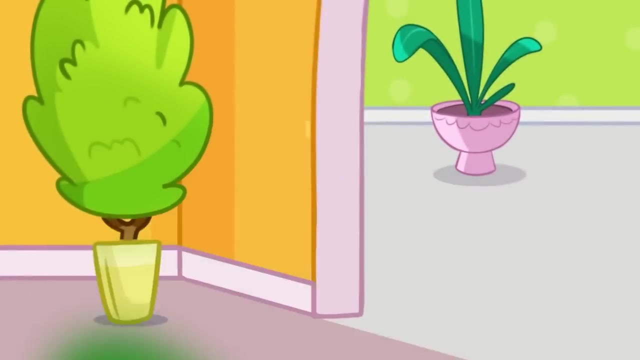 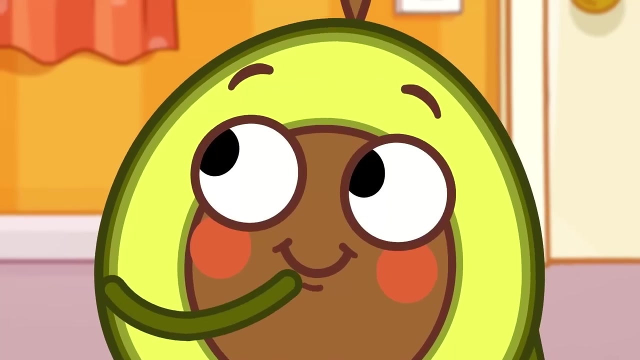 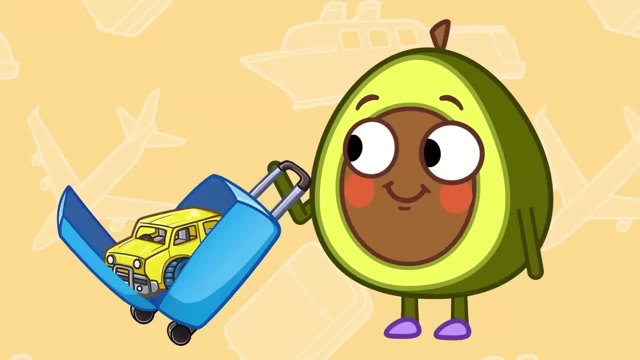 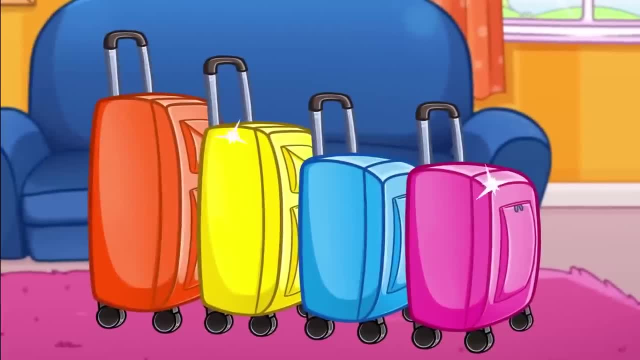 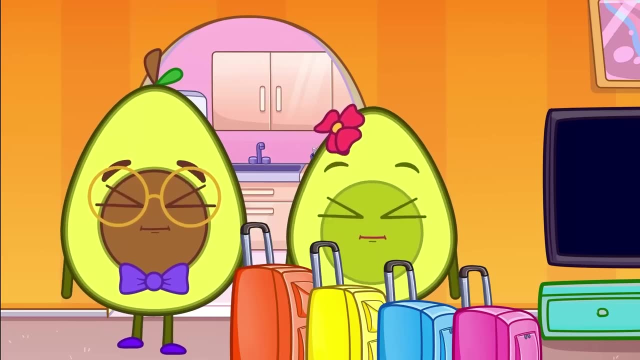 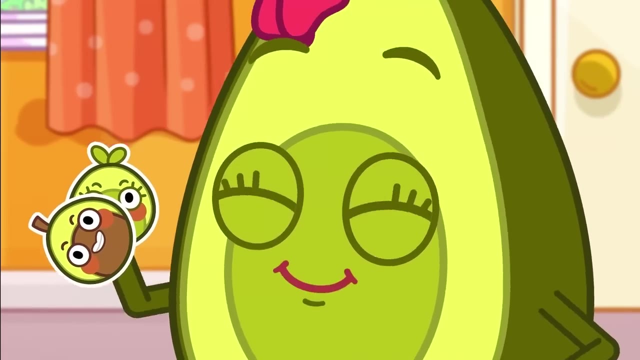 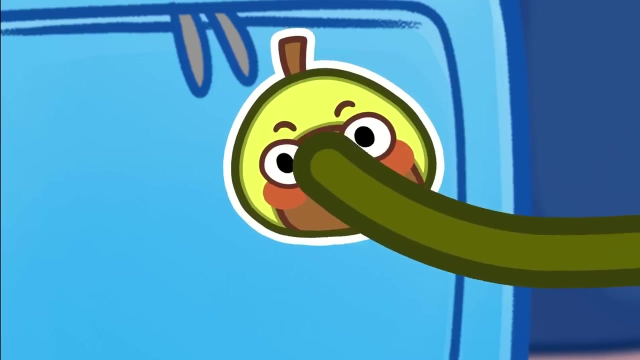 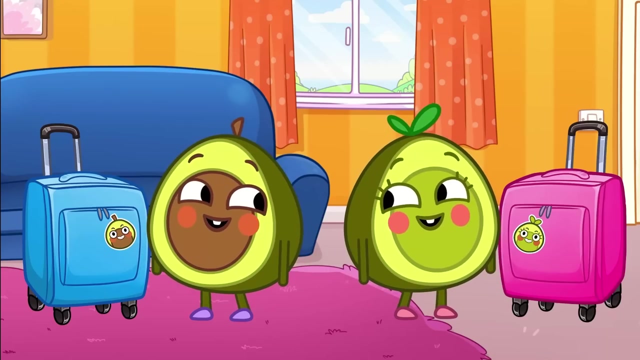 Good job, Pit. The suitcases are finally packed. Hmm, there's one thing left to do. Oooh, Put the stickers on your suitcases so you can easily find them at the airport. Hmm, I wonder what's in Daddy's suitcase? 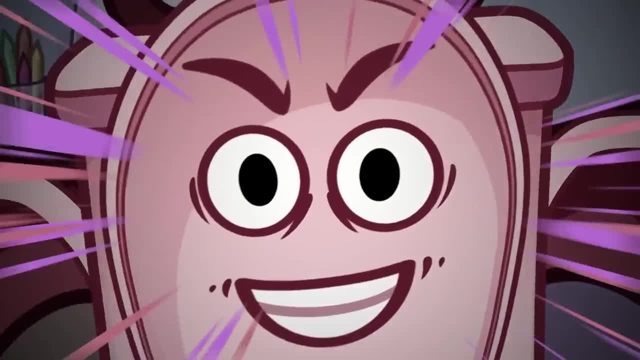 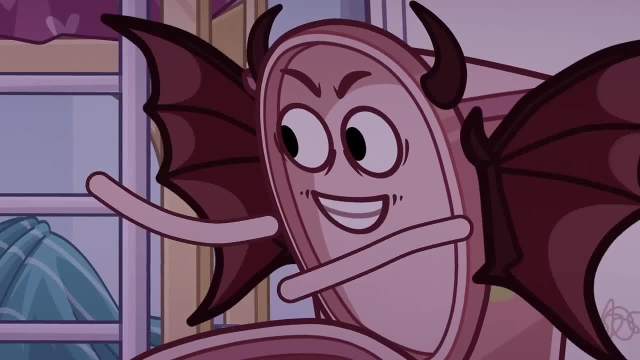 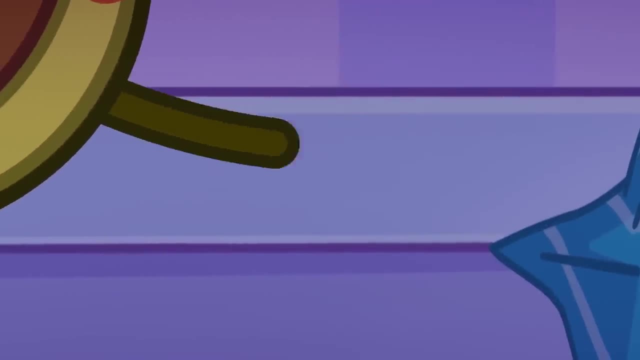 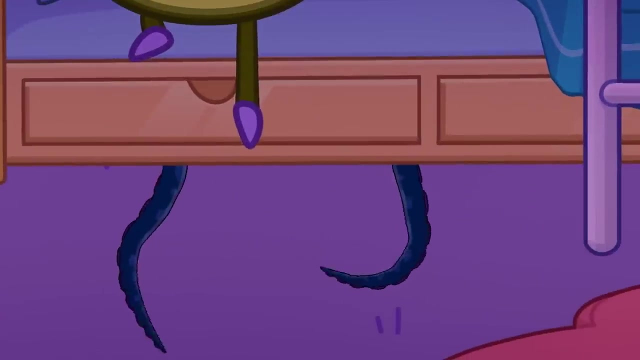 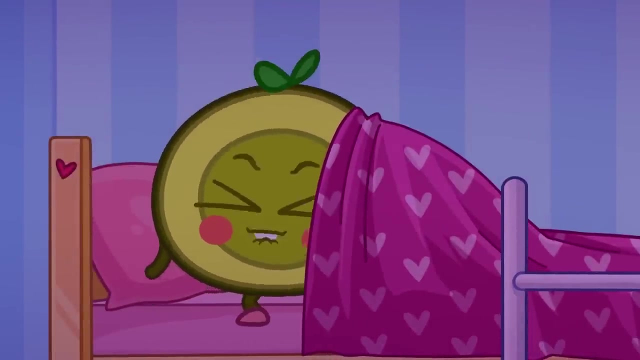 Oh, Pit and Penny. Oh no, Pit wet the bed. It's okay, Pit, It was just a bad dream. Pit needs to use the bathroom, But he thinks there are monsters under the bed. You're yelling. You're woken me up. 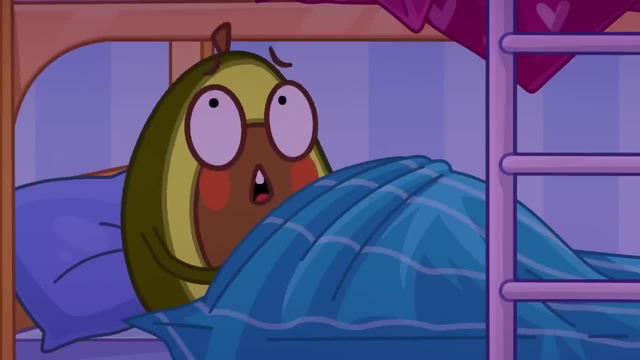 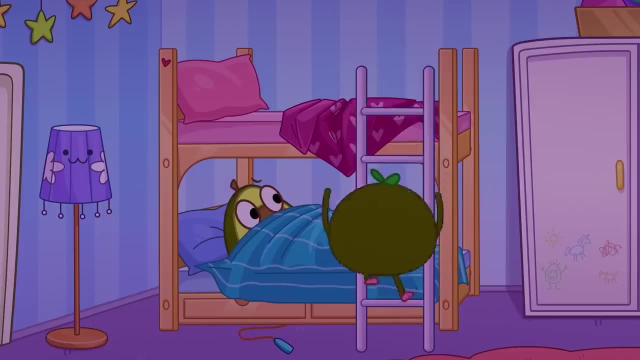 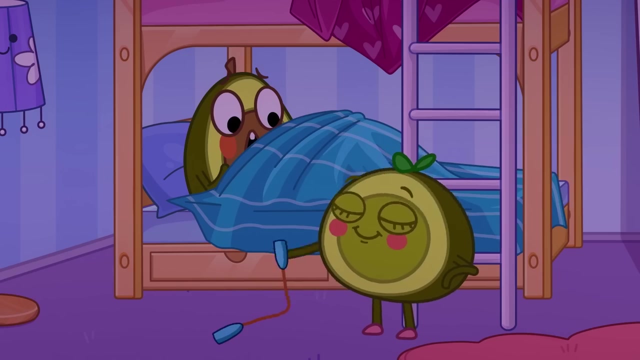 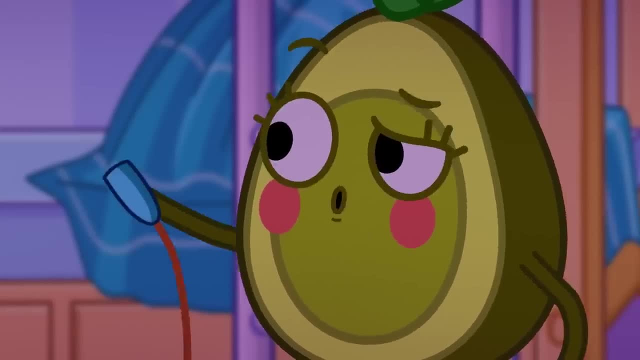 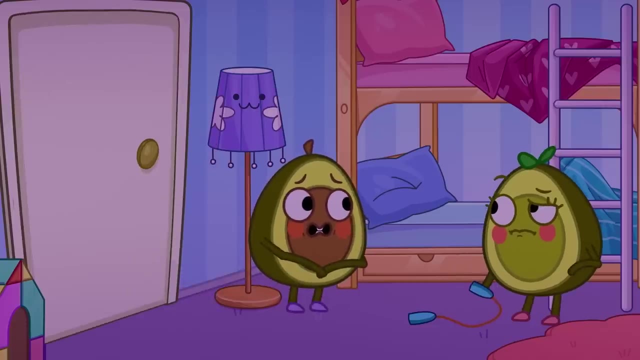 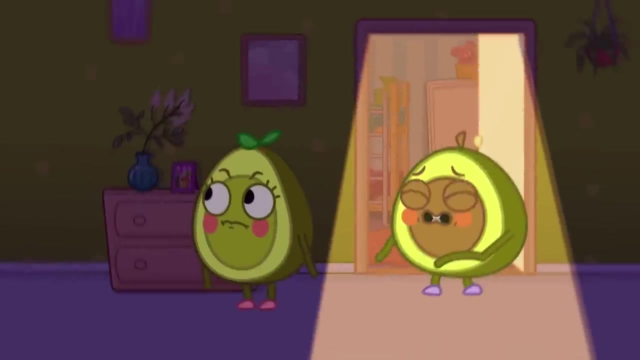 You are going to pee yourself. You are going to pee yourself. Go to the toilet. The hall is dark and scary. The hall is dark and scary. Can you go with him, Penny? Can you go with him, Penny? Uh-oh, Now Penny's scared. 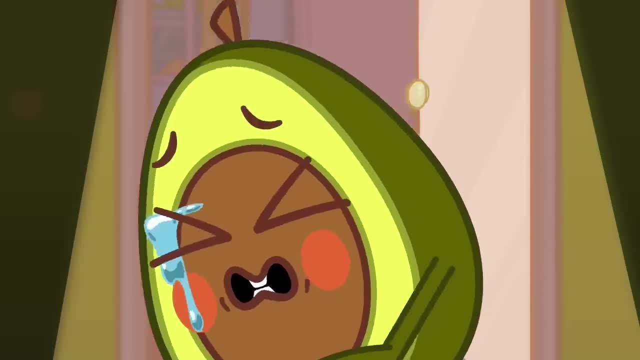 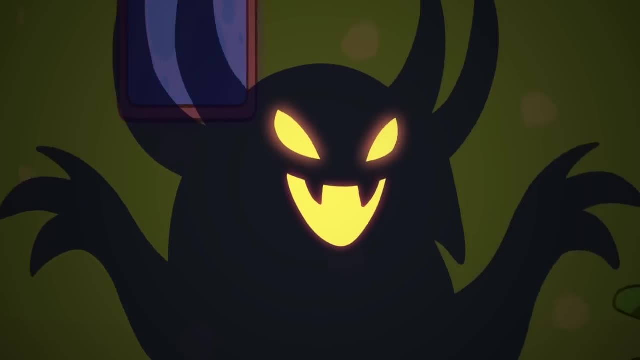 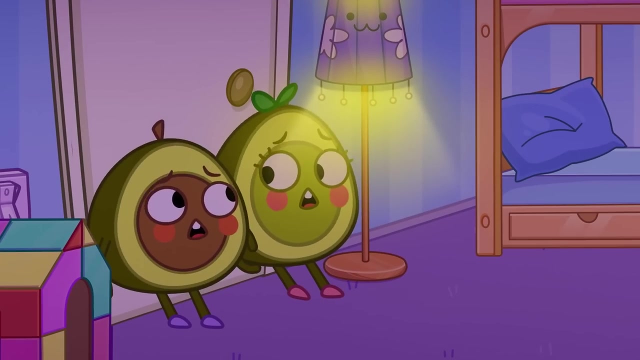 Uh-oh, Now, Penny's scared. Uh-oh, Now Penny's scared. Be brave kids, You can do it. Be brave kids, You can do it. Is that a monster? Is that a monster? Now? what will Pit do? 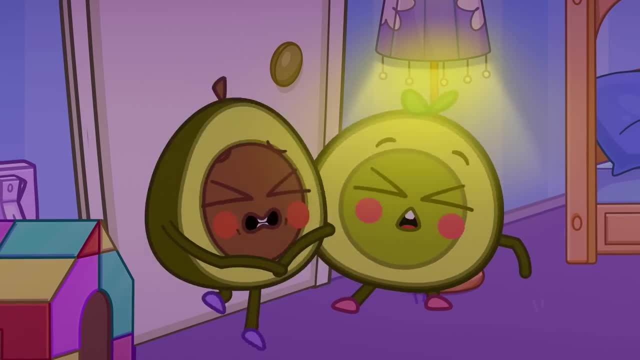 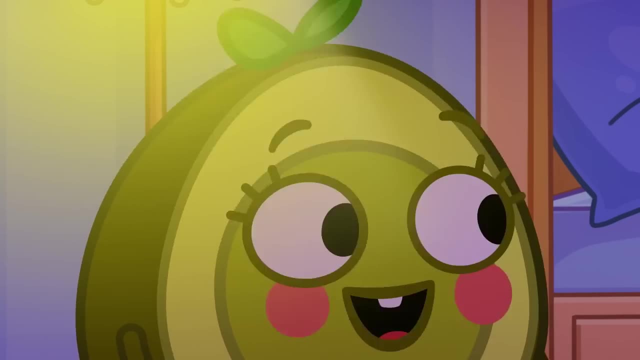 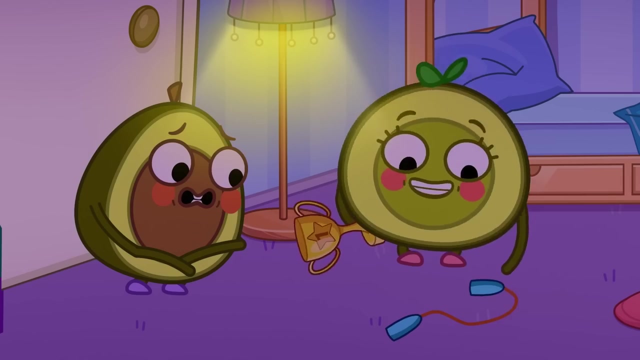 Now, what will Pit do? Now, what will Pit do? Penny, Do something. I can't stand it anymore. It's not funny. It's not funny. Pit needs a real toilet. Get the jump rope, We'll catch him. Get the jump rope, We'll catch him. 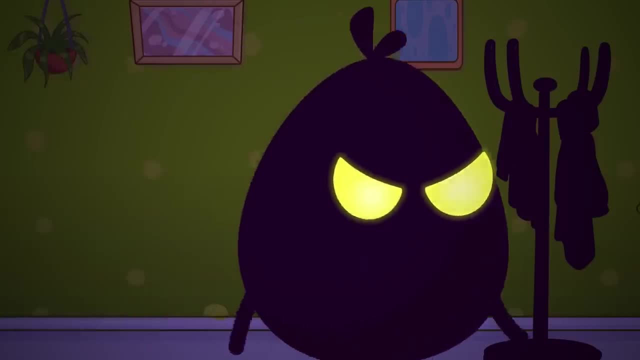 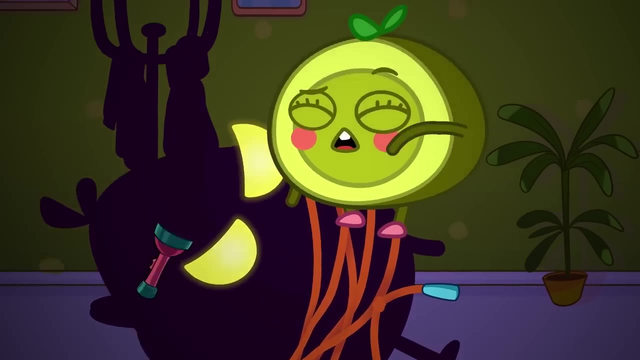 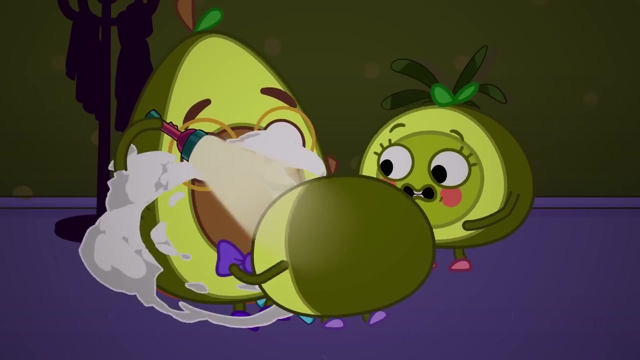 Get the jump rope, We'll catch him. Here comes the monster. Here comes the monster. We have caught it. We have caught it. Wait, That's not a monster. Wait, That's not a monster, It's Daddy. It's Daddy. 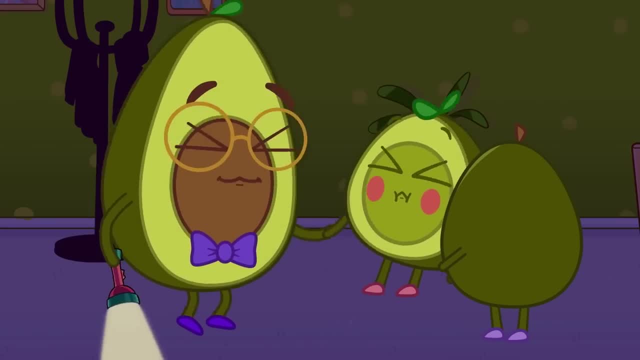 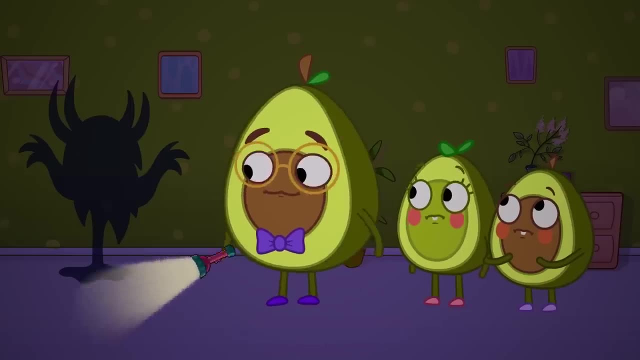 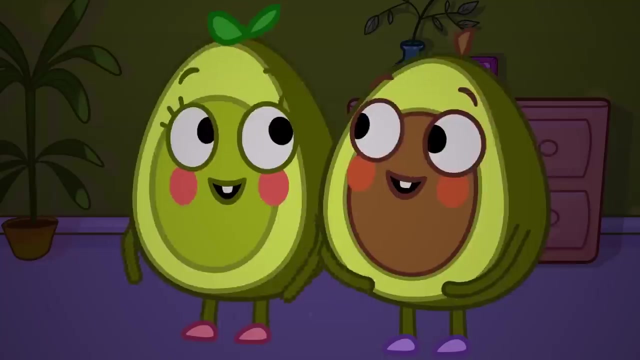 Sorry Daddy, Sorry Daddy, We saw it. That was a monster. That was a monster. Let's see what it really is. It's just a coat rack. It's just a coat rack. Monsters are not real. Monsters are not real. 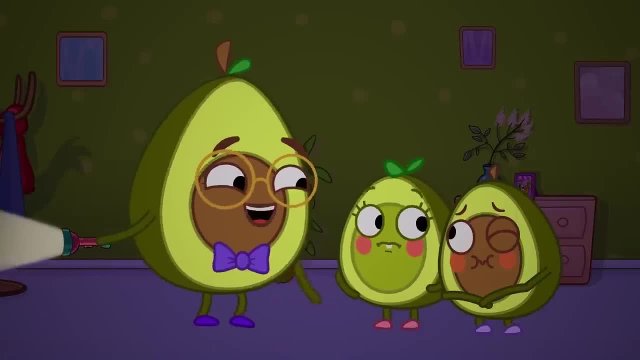 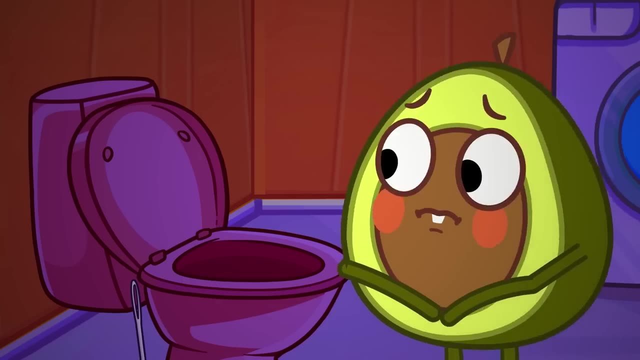 Pit really needs the toilet now. Pit really needs the toilet now. I think it's time to pee. I think it's time to pee In the dark. In the dark, the toilet seems scary. the toilet seems scary, But there's nothing. 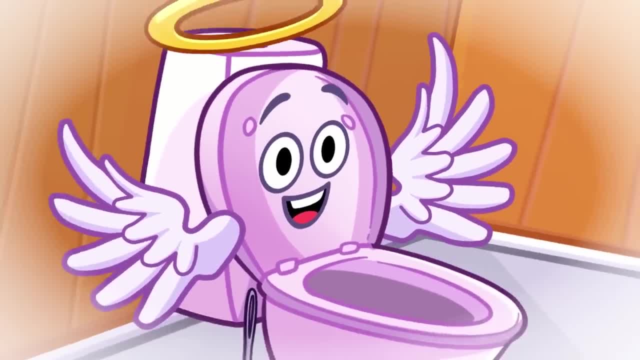 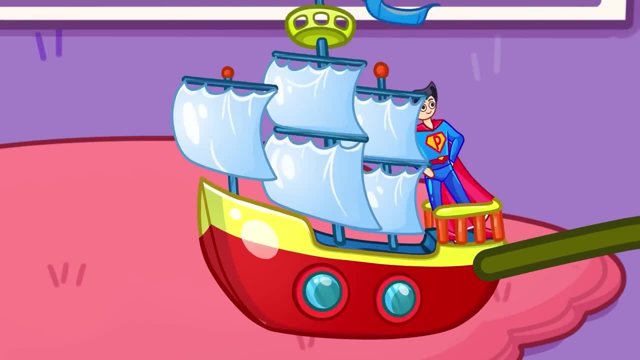 But there's nothing to be scared of. But there's nothing to be scared of. Yay, Finally, Pit feels better. Pit is playing with his super pal toy, Pit is playing with his super pal toy And Penny has a shark. 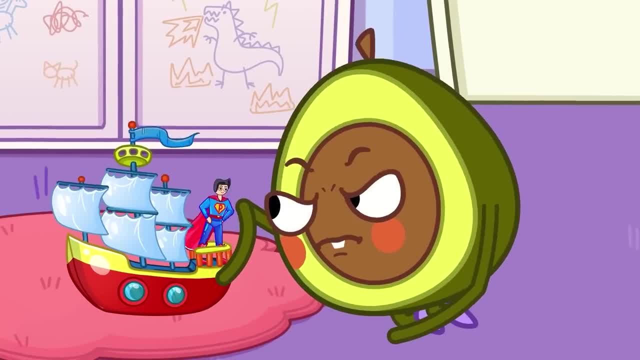 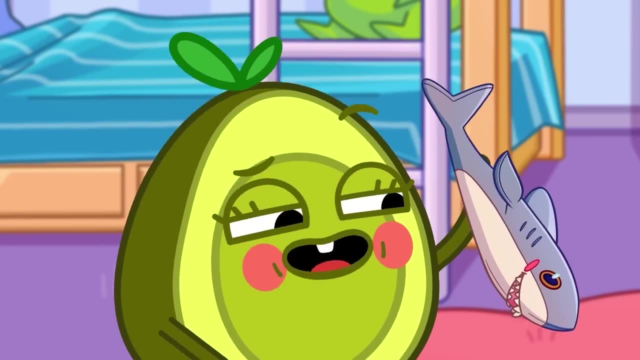 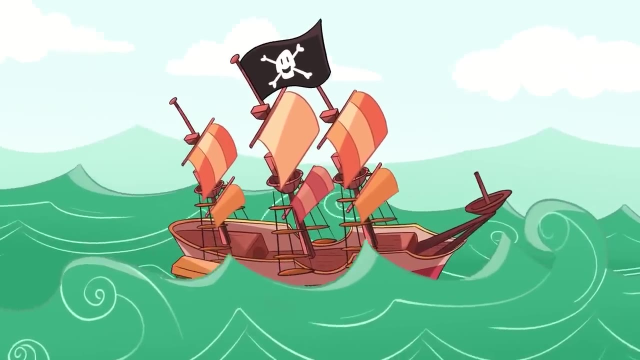 And Penny has a shark. Your shark can eat my superhero. Is that true, Penny? Is that true Penny? No, Baby shark is good. Let's play pretend and see. Let's play pretend and see. Let's play pretend and see. 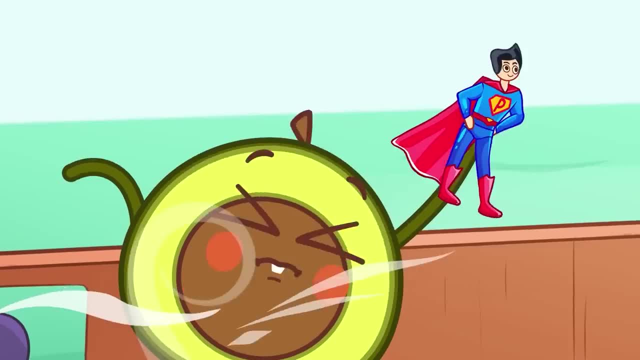 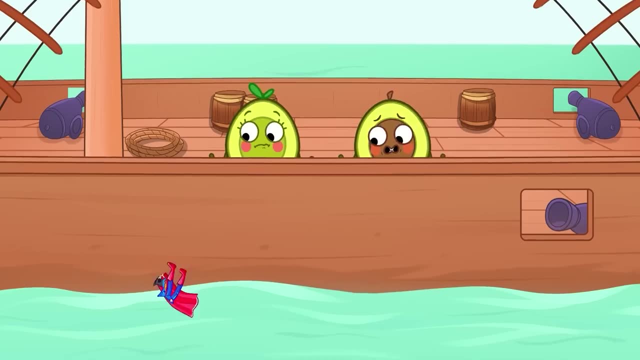 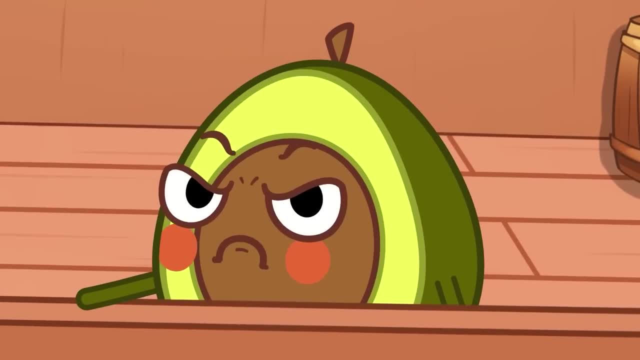 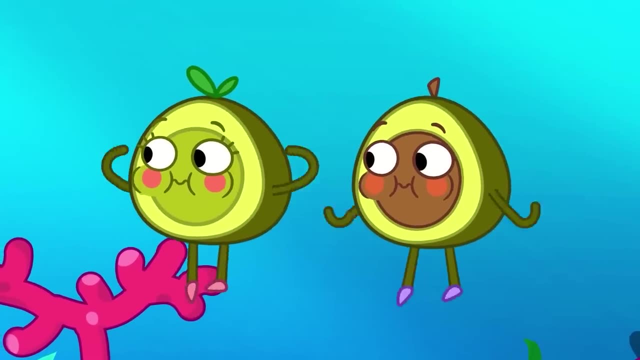 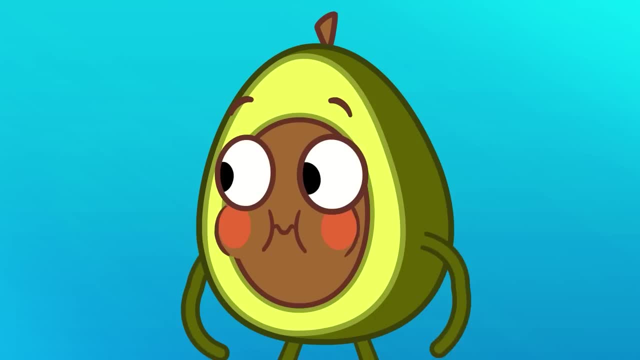 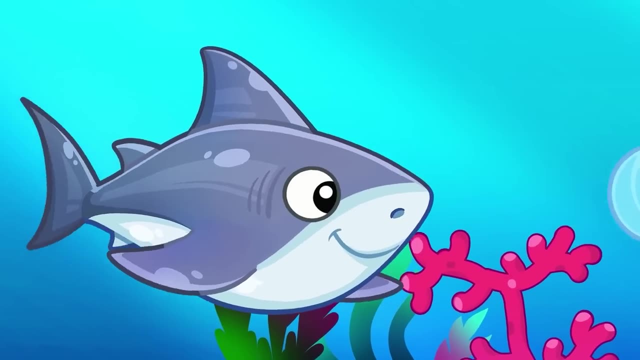 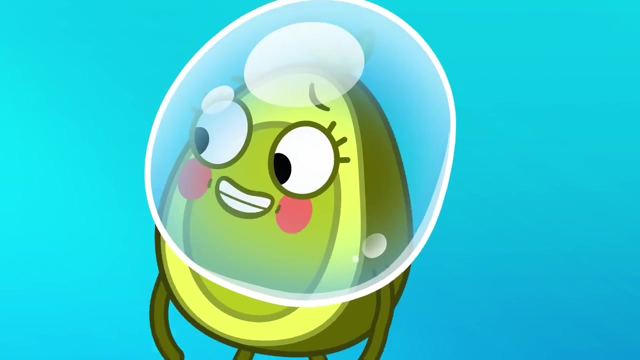 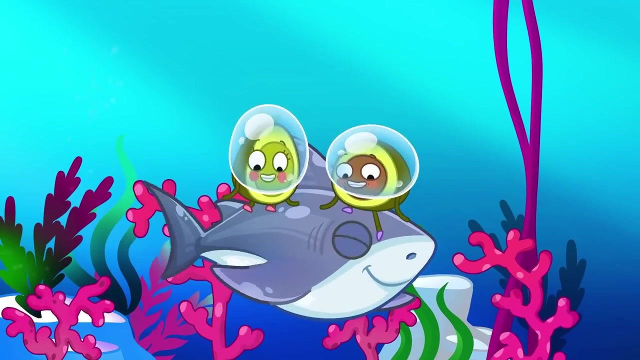 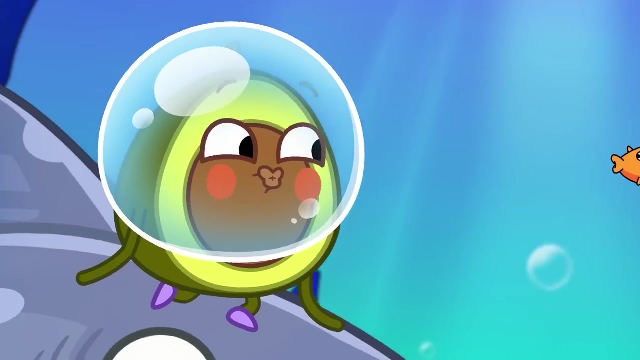 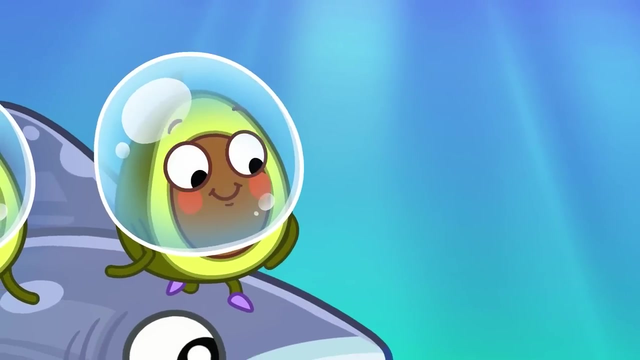 Now Pit and Penny are on a ship. It needs some air. Yes, Thank you, Baby Shark. Baby Shark, please help us find Big's toy. Look, It's a pufferfish. What's that? My toy is there. 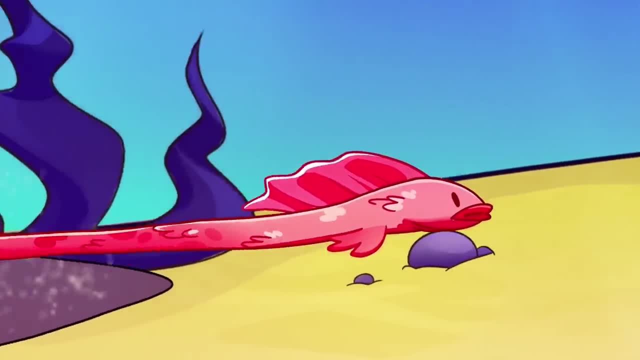 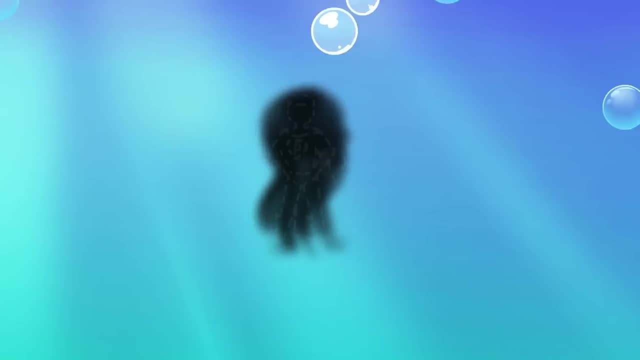 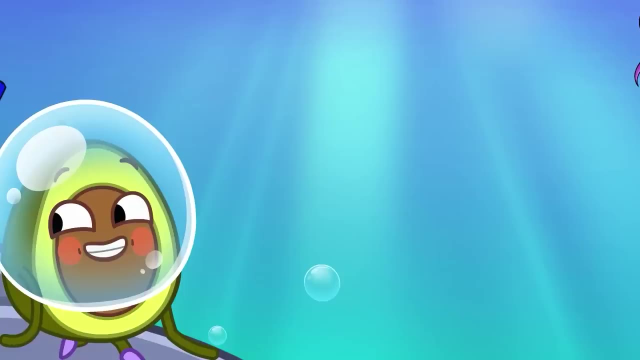 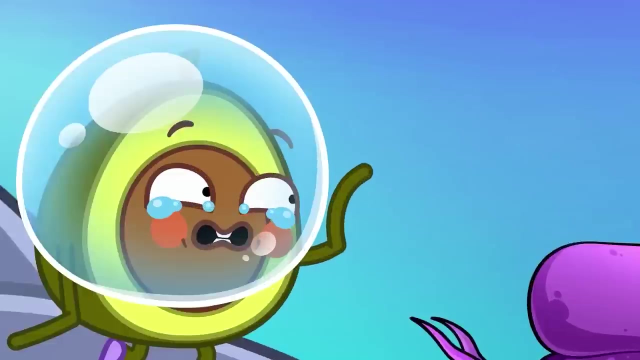 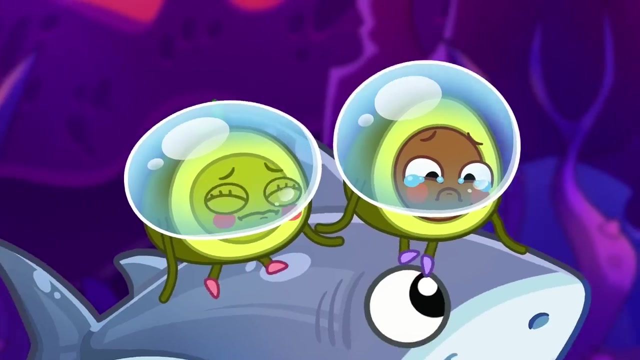 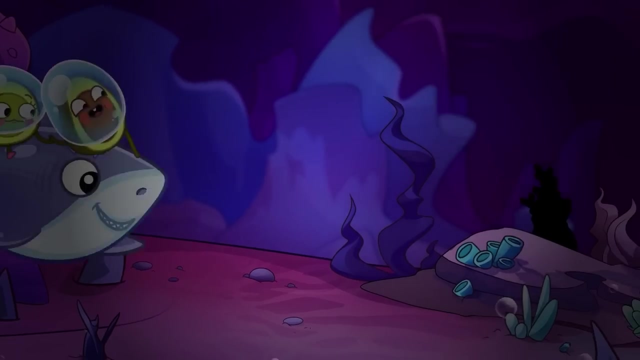 Nope, It's just a fish. Maybe that's Big's toy. What is this? It's a jellyfish. Careful Jellyfish can sting you. I see the toy. Let's take a closer look. I can't see anything here. 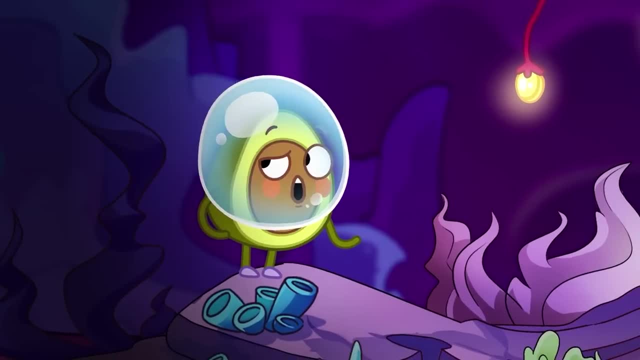 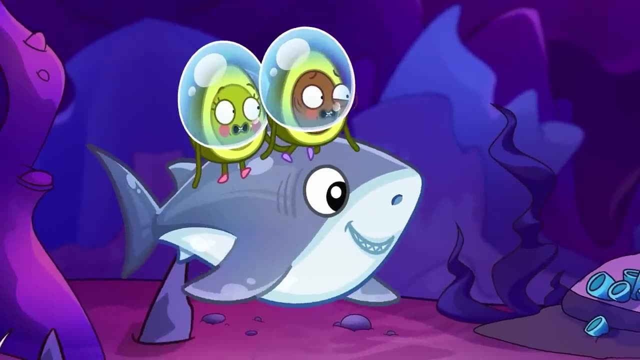 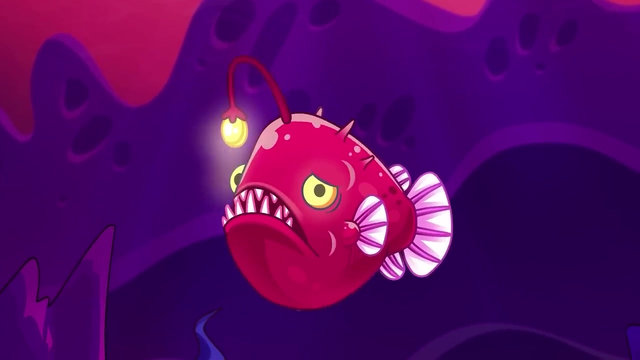 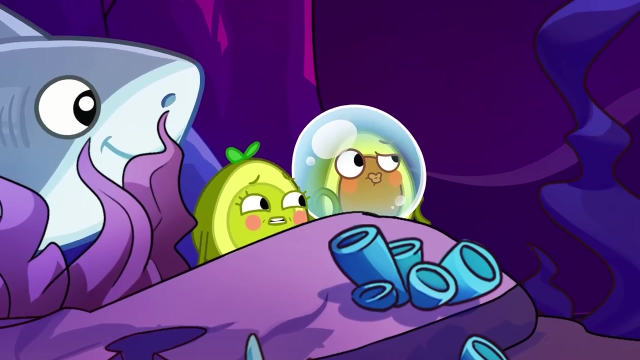 Oh, it's a piece of coral. This is not my toy. Where did that light come from? It's an anglerfish. No, No, No, No, No, No. It has an upset tummy. He's eating something wrong. 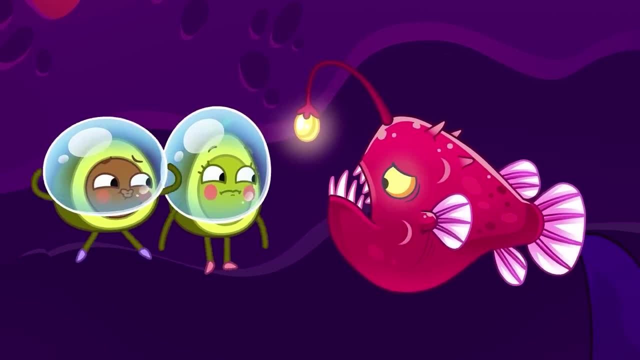 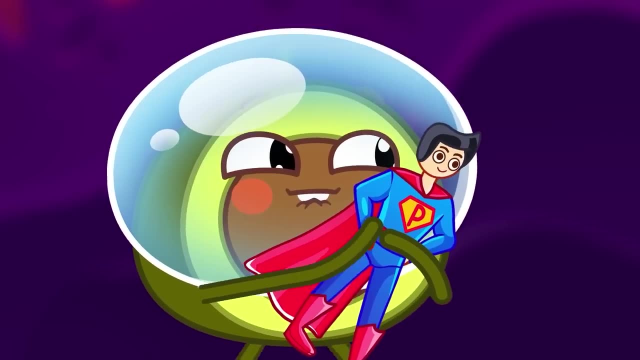 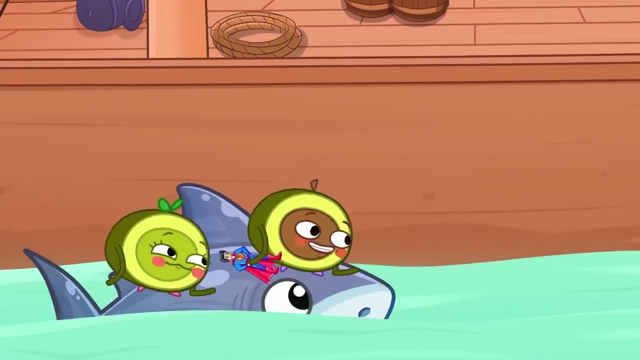 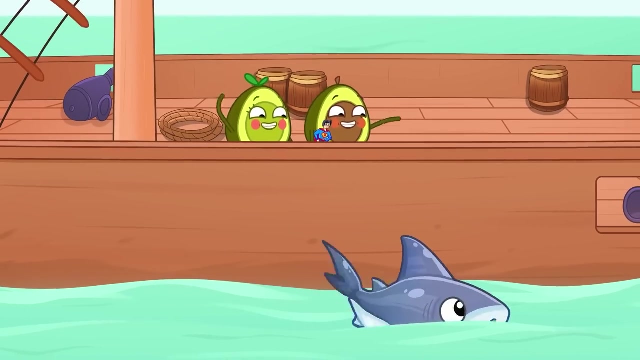 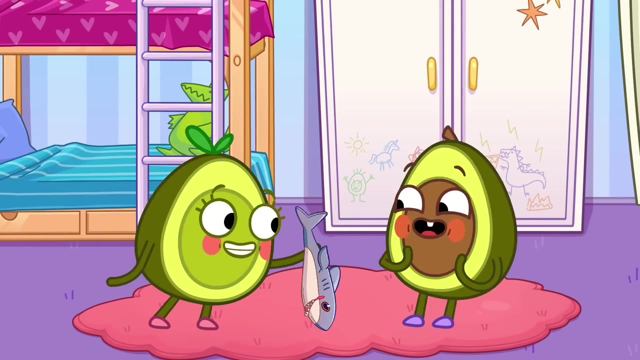 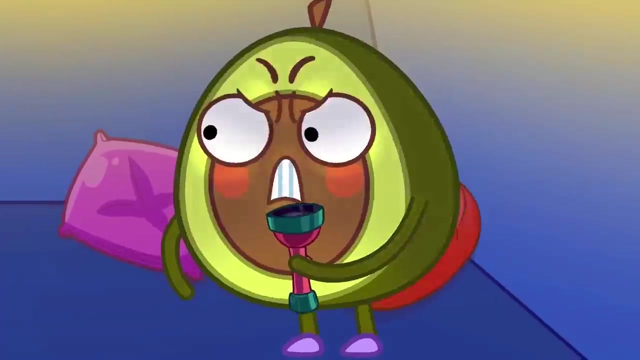 Look what he ate. This is my toy. This is my toy. This is my toy. Don't forget to thank Baby Shark. Thank you, Baby Shark. See Pit, Baby Shark isn't scary at all. Pit and Penny are in their tent. 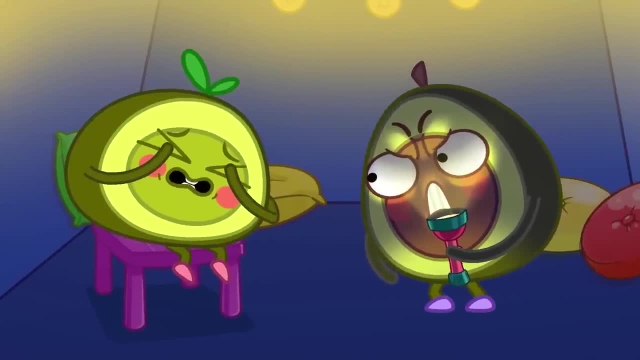 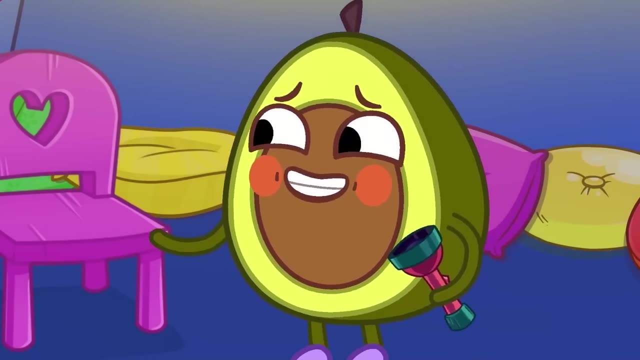 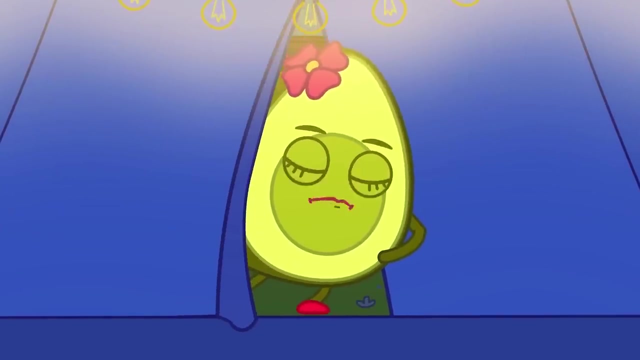 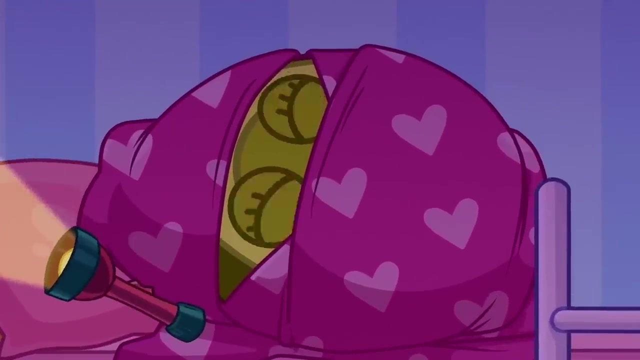 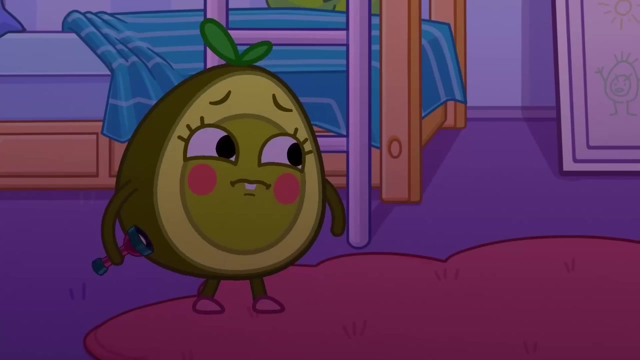 Pit is telling ghost stories. Penny is scared. That's not very nice, Pit Kids, it's time to sleep. Penny is cozy in bed. The storm has opened her window. No, It's okay, Penny, You're so brave. 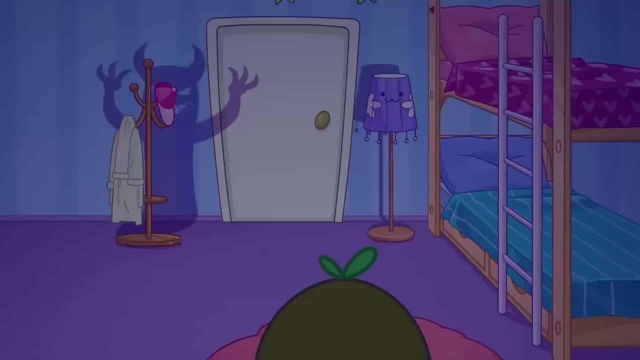 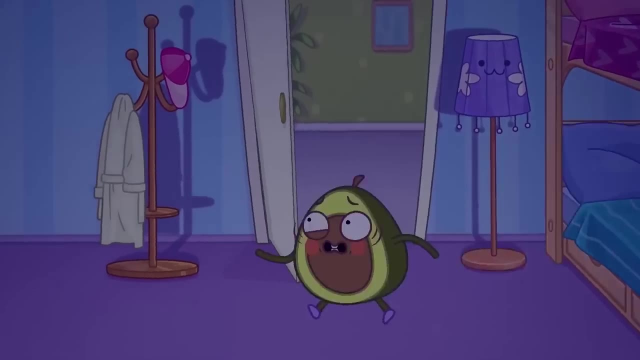 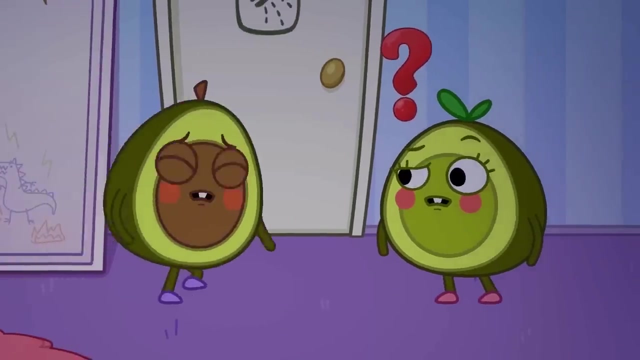 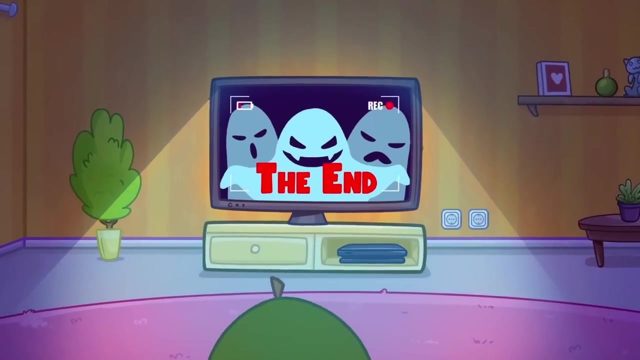 That's better. Now the window is closed. Penny thinks she sees a monster, But there's nothing there. What's wrong, Pit? Now it's Pit's turn to be scared. Pit was watching a scary movie And he cried And he got frightened. 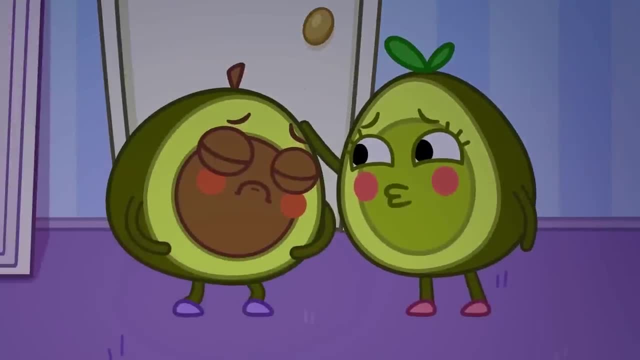 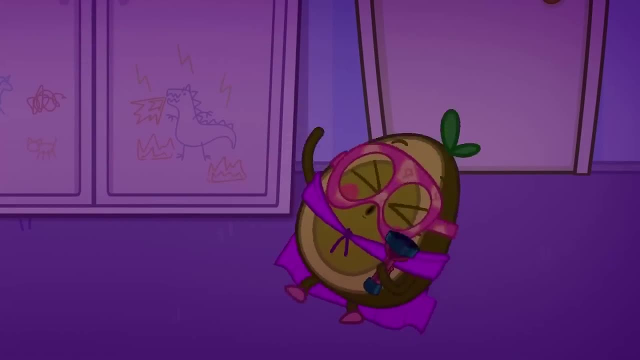 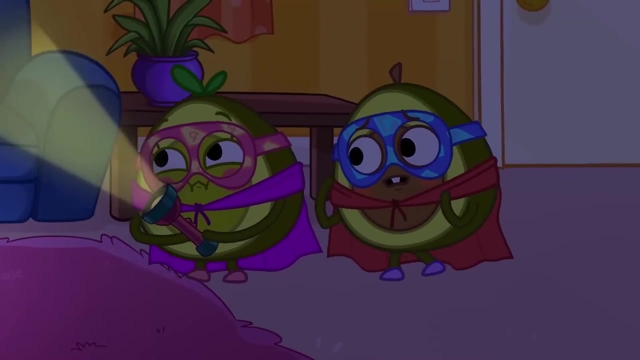 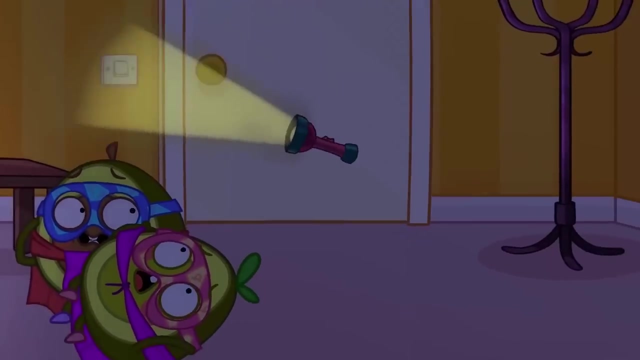 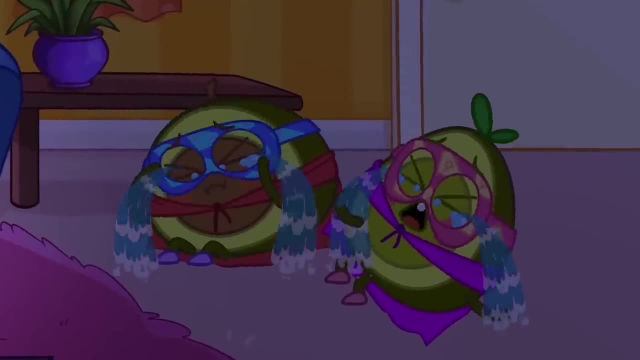 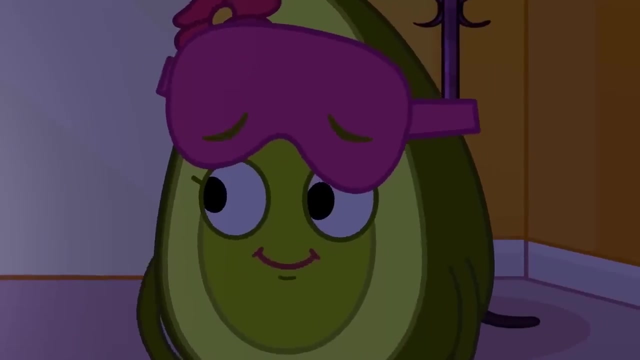 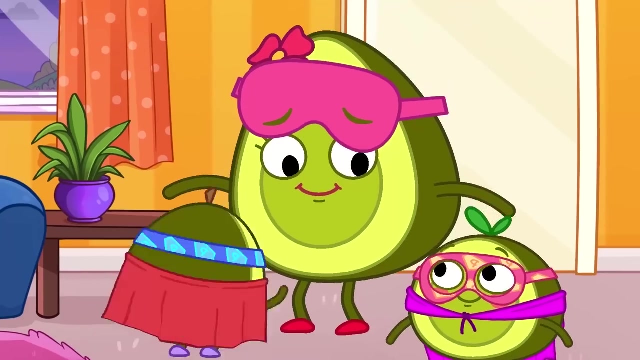 Now the room is dark. Now the room is dark and scary. Mommy is here to save the day. Mommy turns on the lights. It looks like the monster was just a tree branch Pit and Penny are at the amusement park. Oh, wow, a. 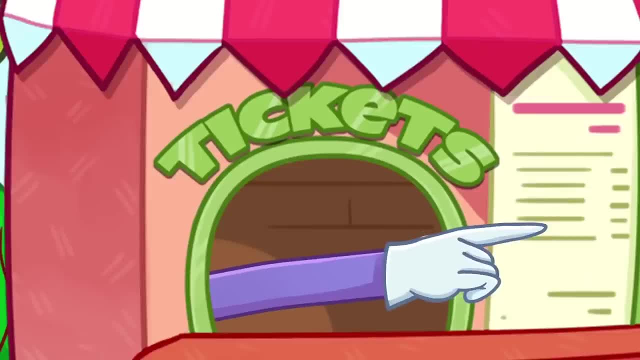 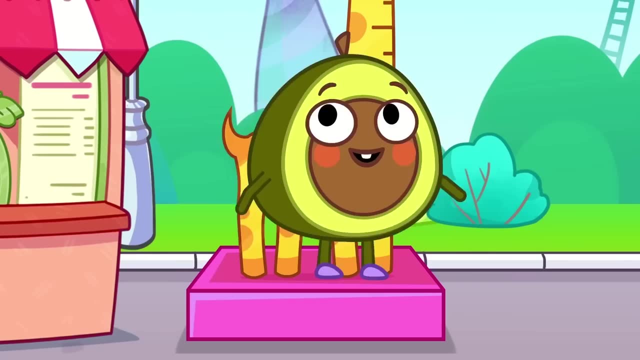 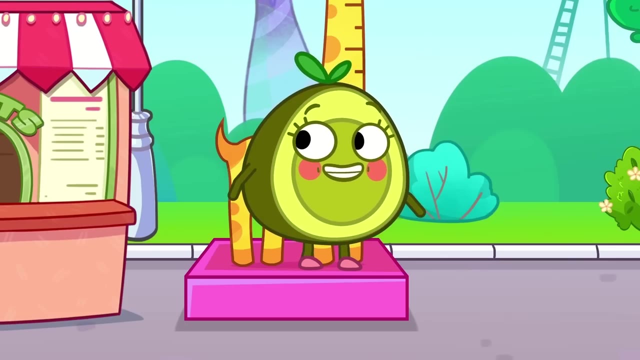 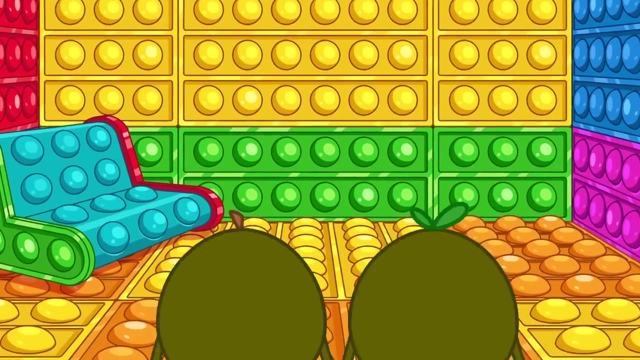 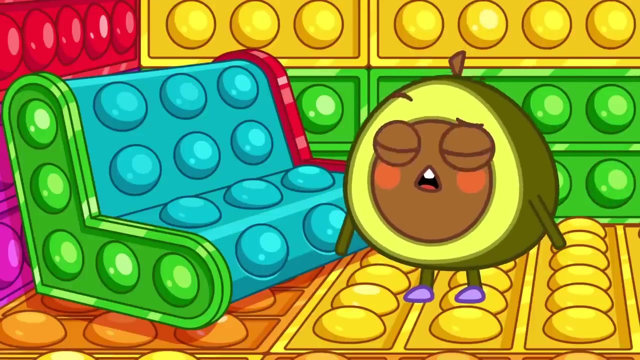 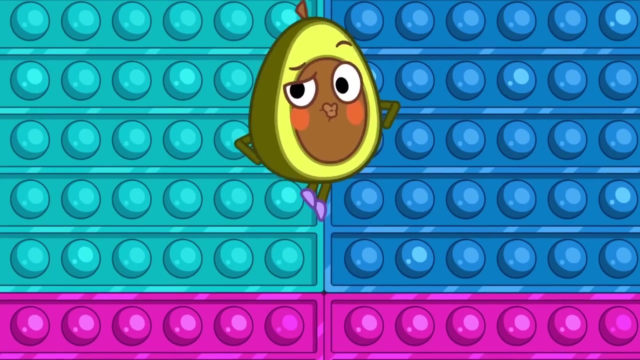 poppet house. Pit measures himself against the giraffe. Pit is big enough to go into the poppet house. It's okay, Penny, you can go in too. Have fun, Pit and Penny. Penny presses all the bubbles. The bubbles are soft and squishy. Wow, look at that bubble. Oh no, Pit is trapped in. 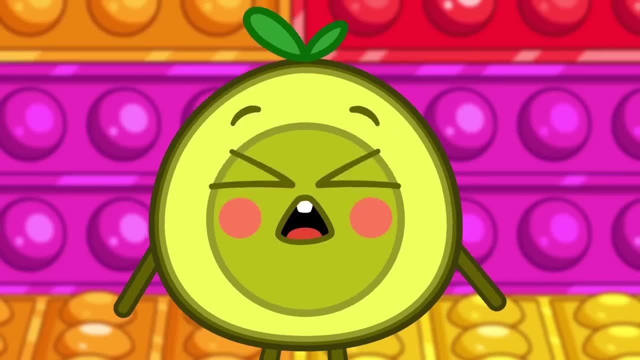 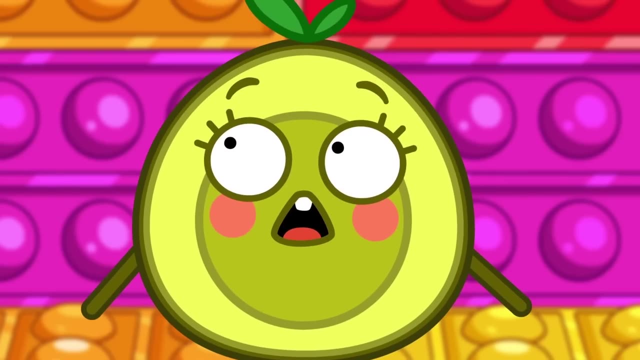 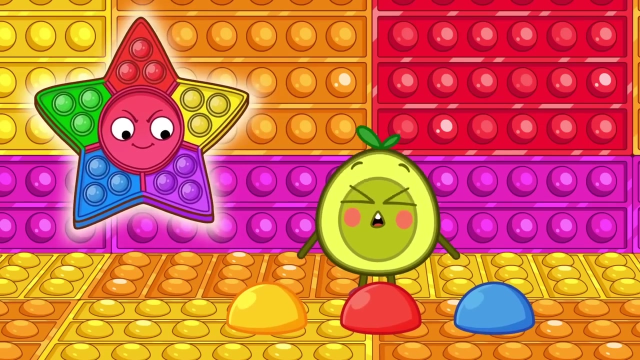 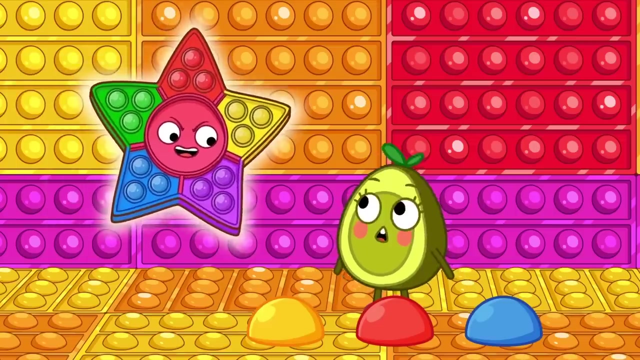 the giant bubble. Penny, you need to help Pit Look out To save your brother. you have to guess all the colors. Don't worry, Penny, you can do this. What color is the sun? That's not right. Try again. 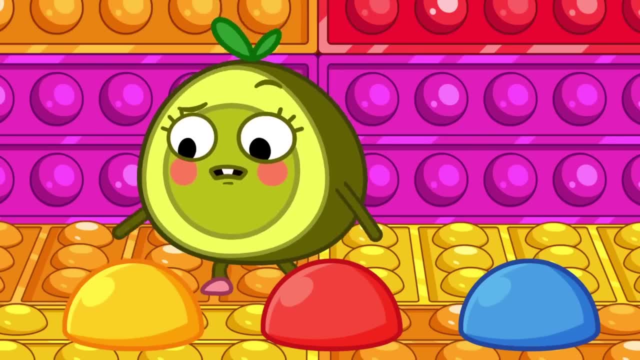 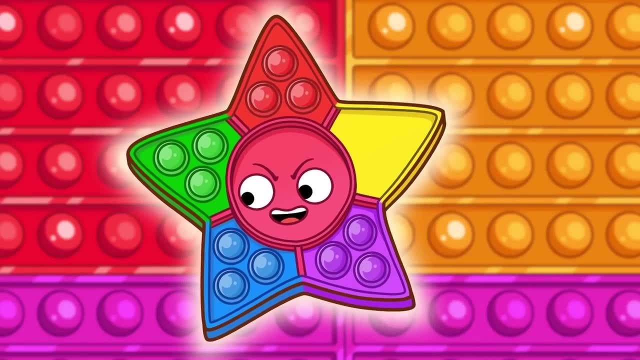 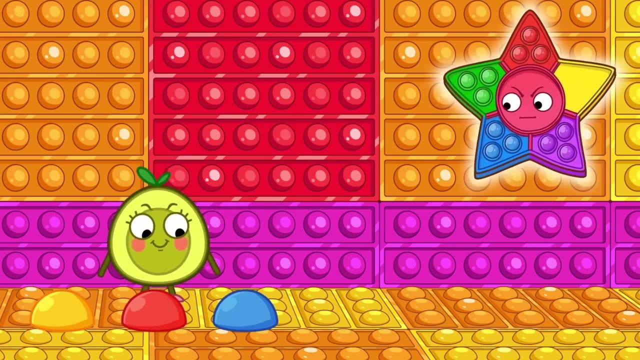 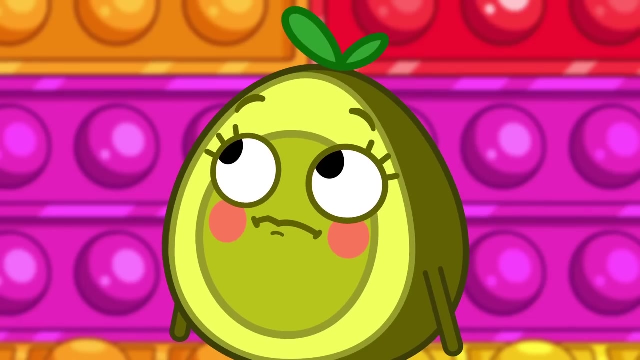 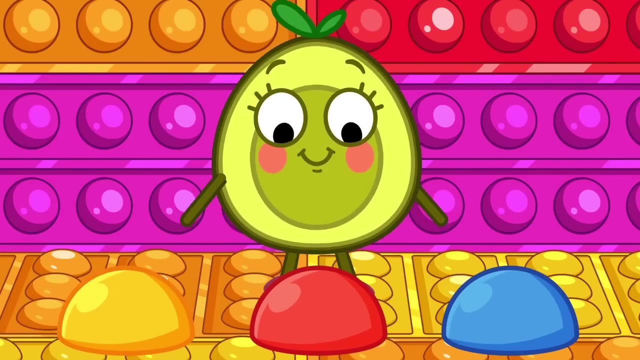 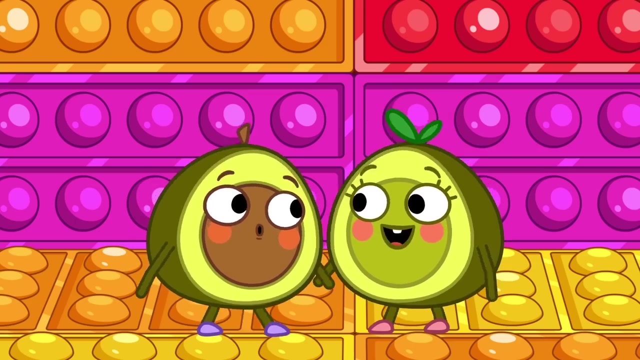 Penny Yellow. What color is the sea? Blue, What color am I? Hmm…, Huh, Hmm…. Penny is thinking Red. Okay, you win. Oh, Oh, Oh. Thank you for your help, Pit and Penny. see more poppets. 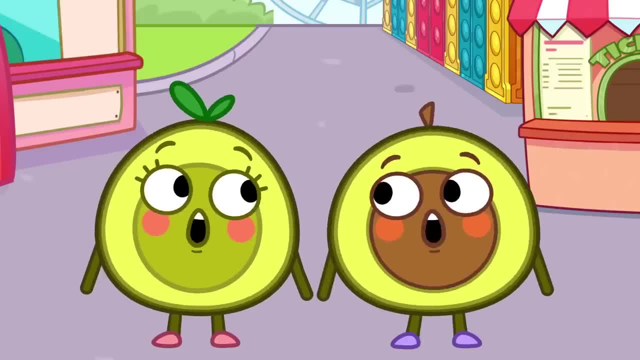 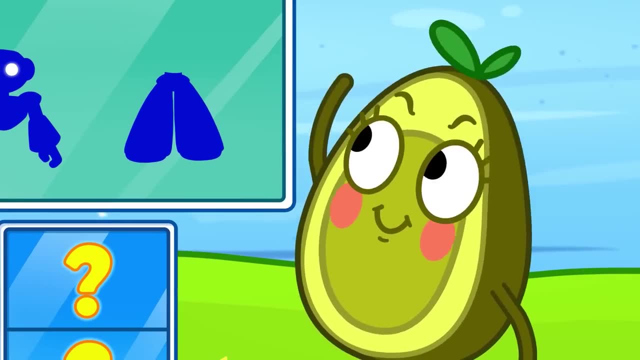 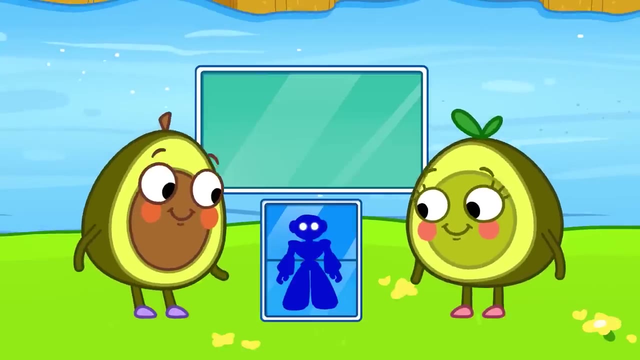 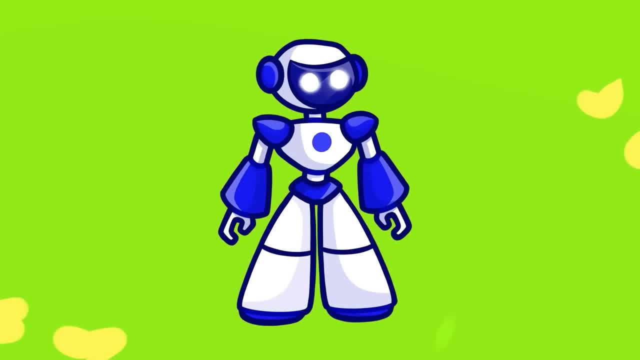 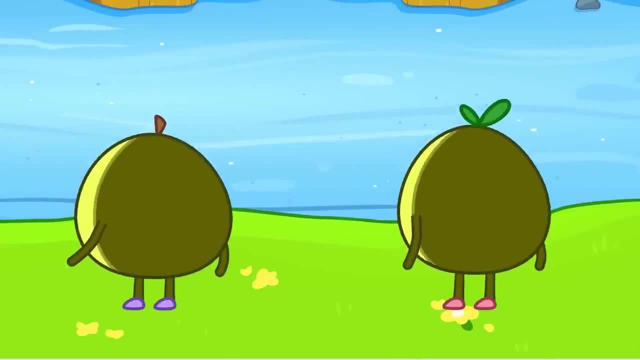 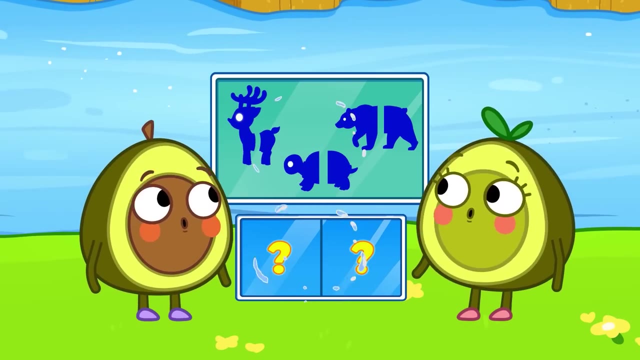 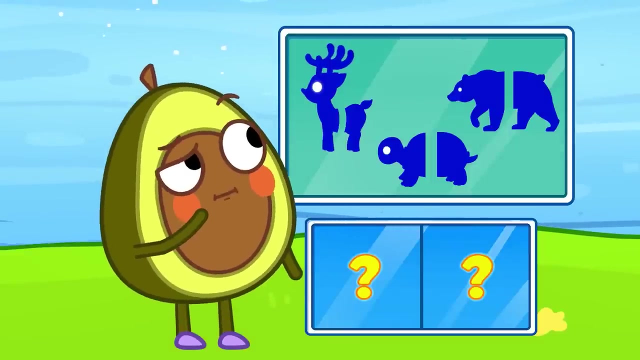 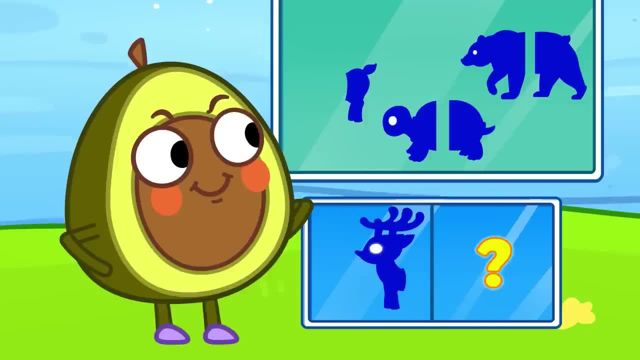 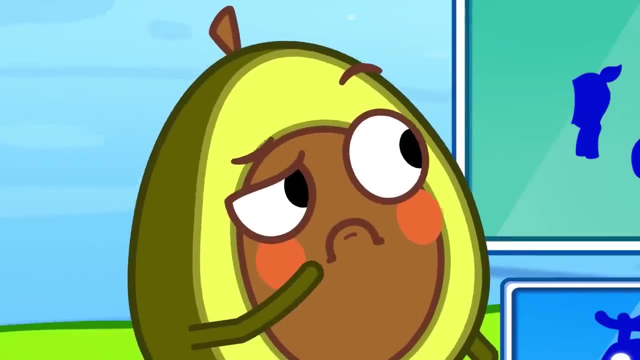 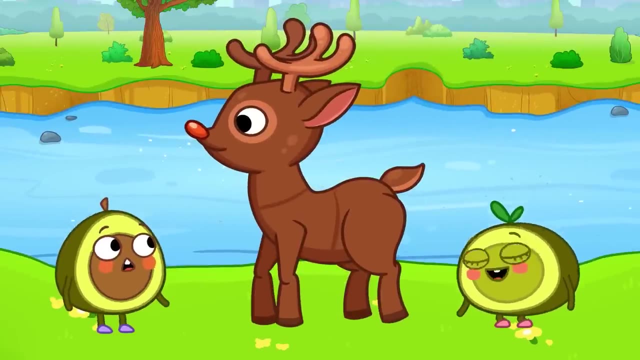 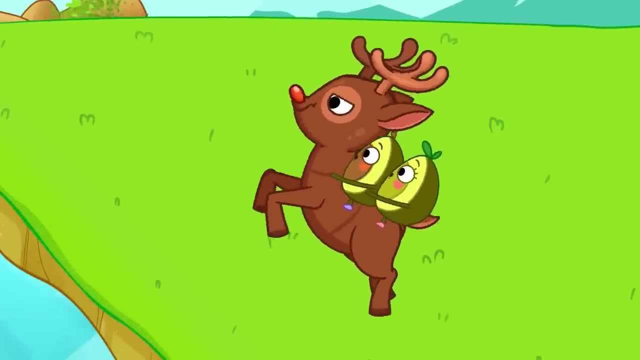 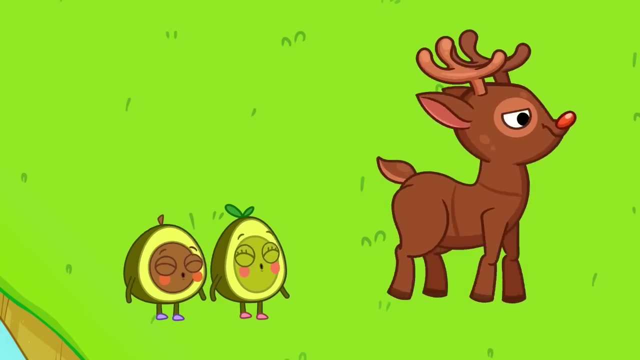 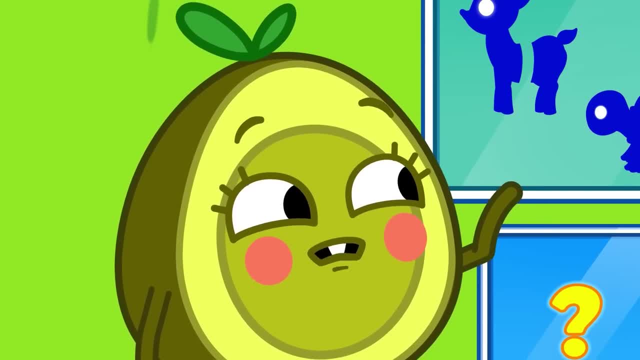 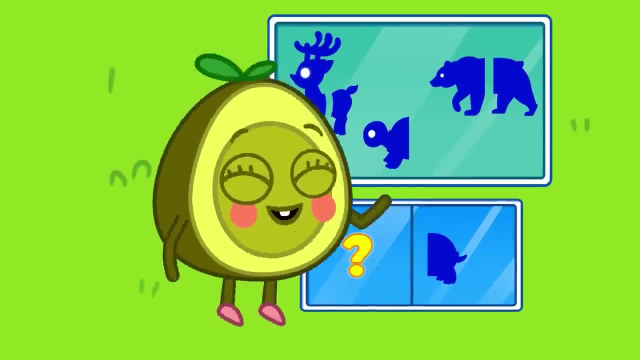 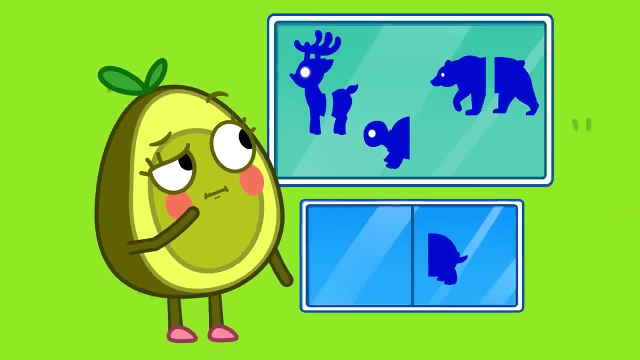 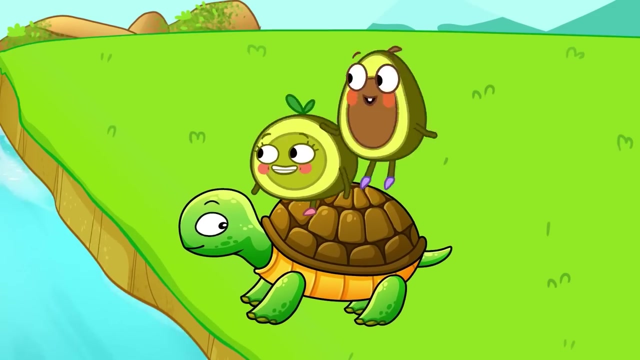 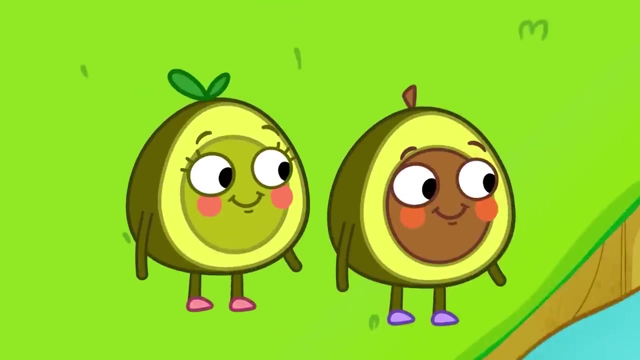 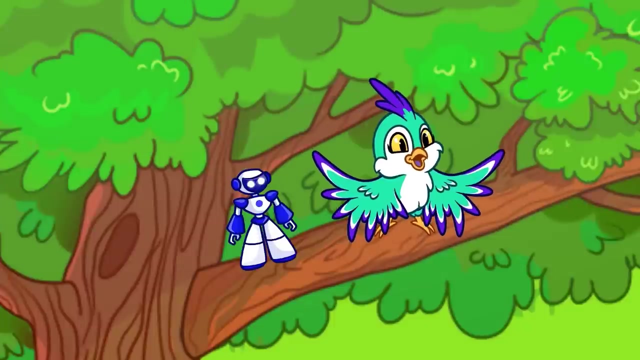 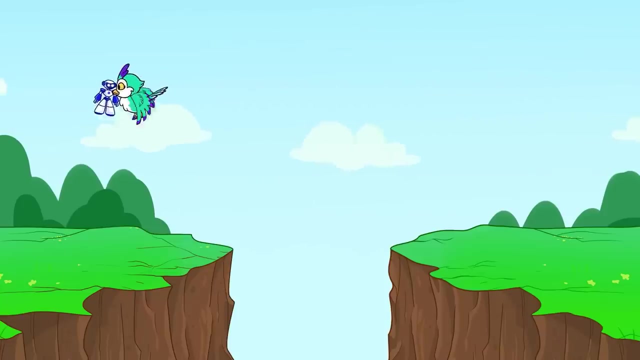 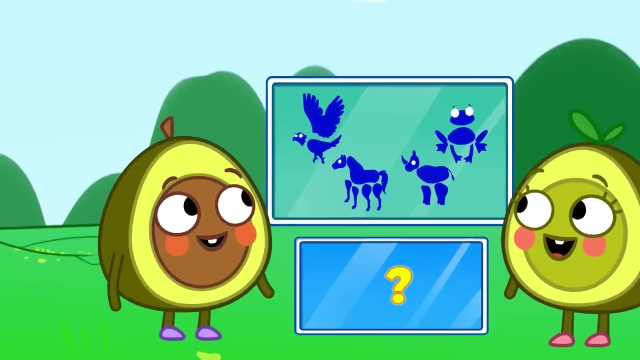 I know who will help us cross the river. That's not a match. Try again. Penny made a turtle. Turtles love to swim. There's the robot. The bird flew away and took the toy across a cliff. What will help us get over the cliff? 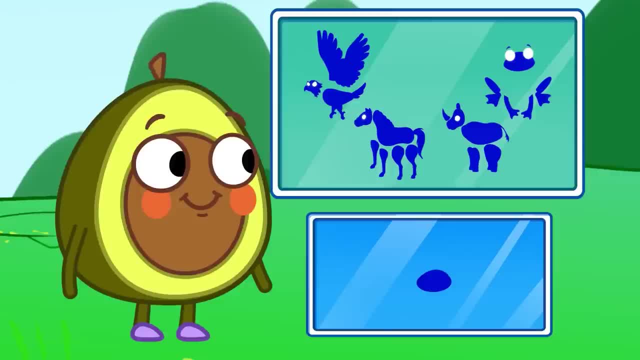 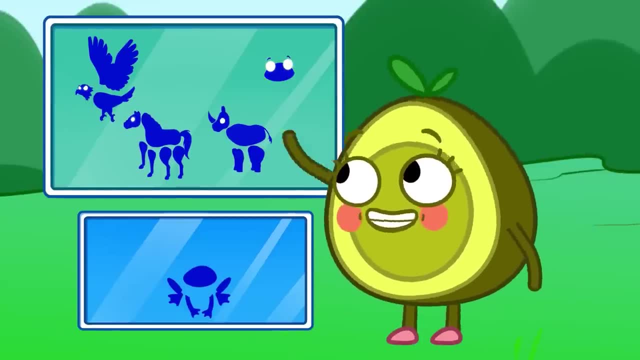 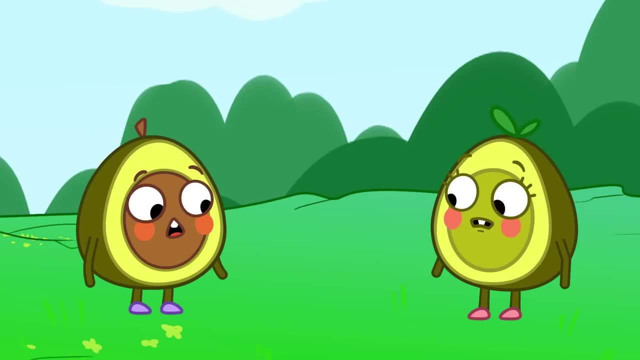 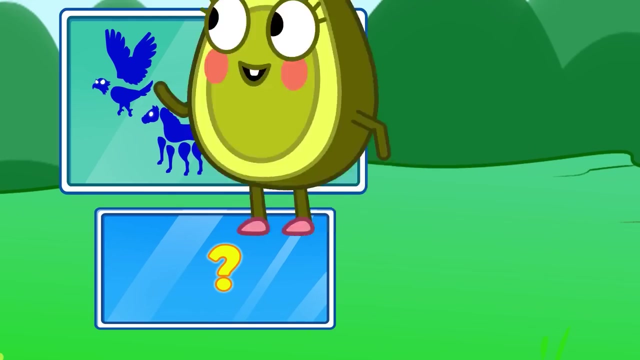 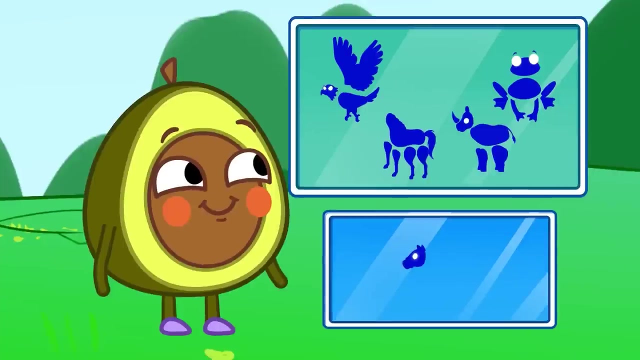 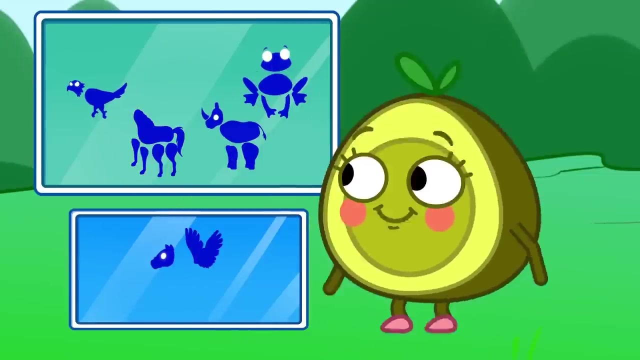 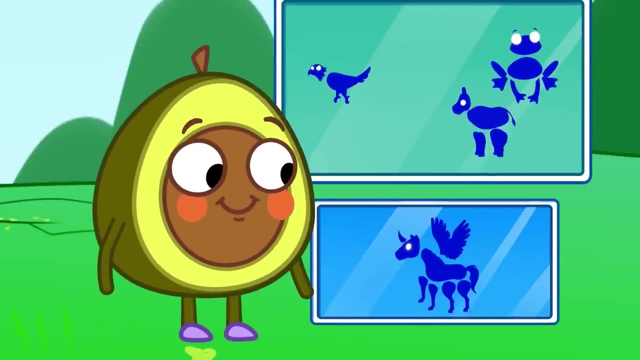 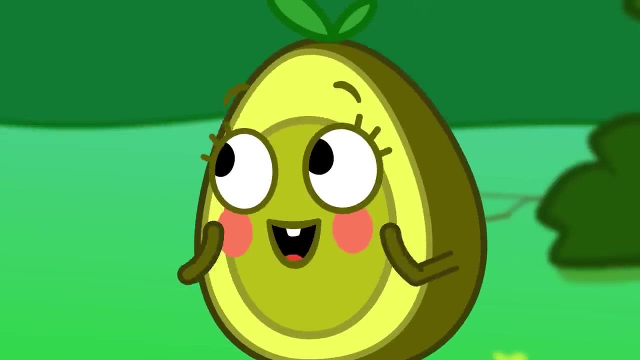 Oh, I wonder what it'll be. It's a frog Pit, and Penny need something bigger. We need a horse. Look One illegal. What an interesting mix. But what is it, Penny, We have made a winged unicorn. 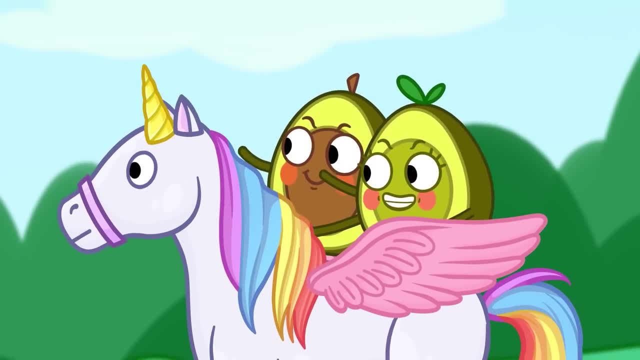 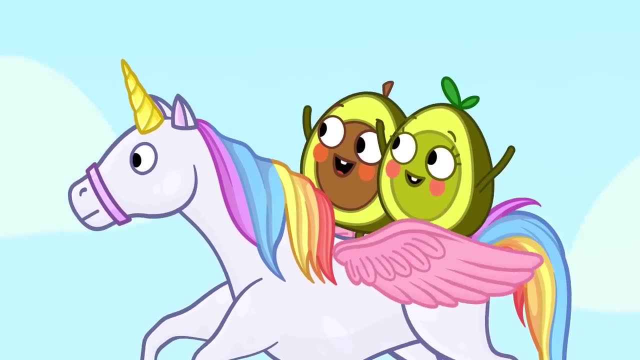 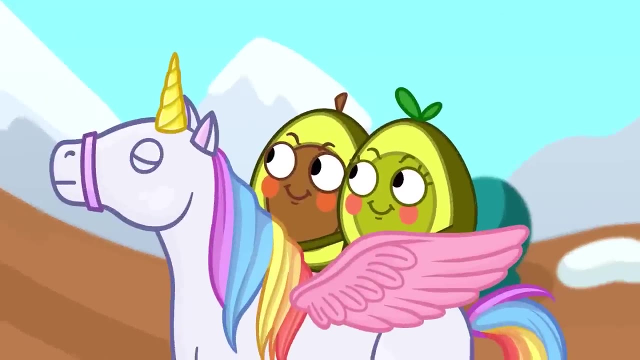 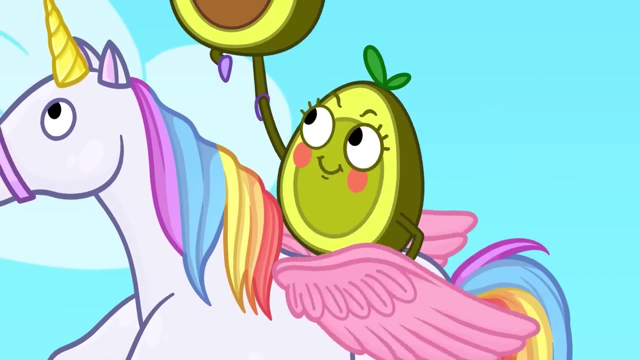 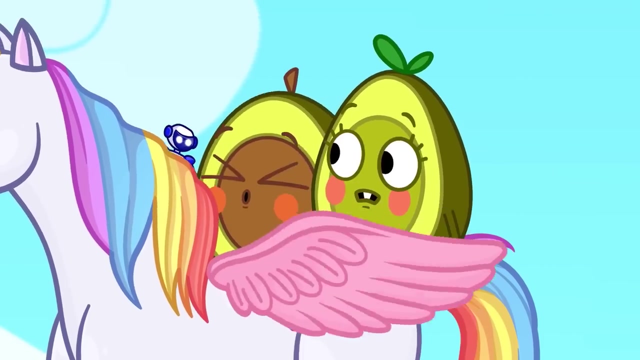 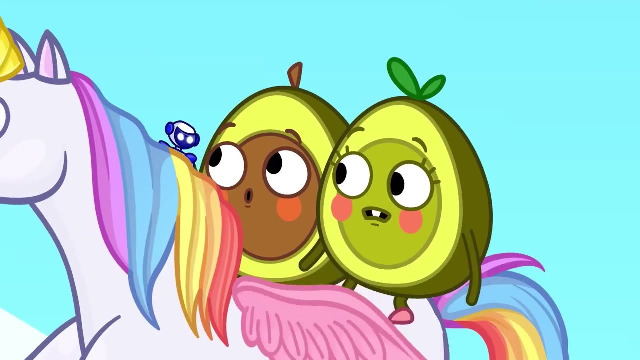 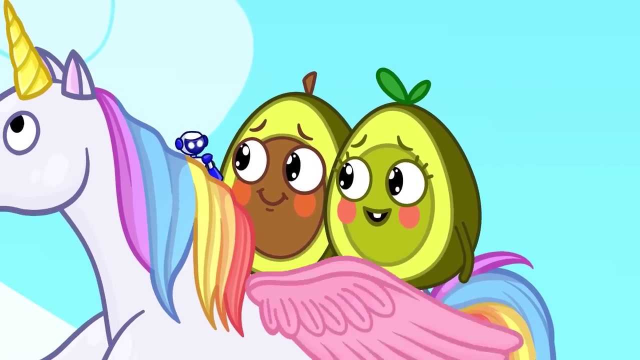 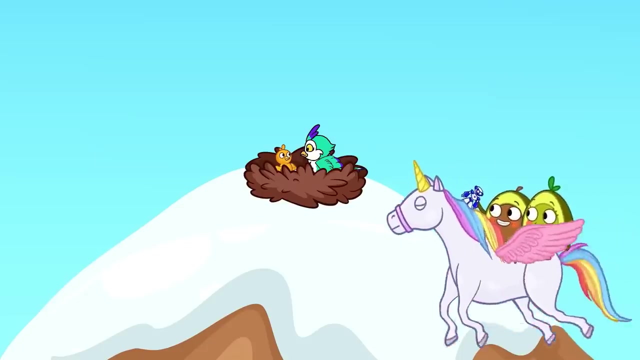 It can fly over the cliff. The toy is up in the nest. Grab it, Pit. Yay, They got their robot back. The egg is hatching And there's a chick inside. The chick needs a toy. Here's a robot for the new baby bird. 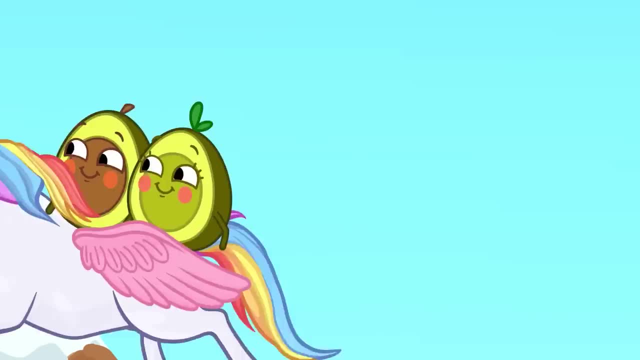 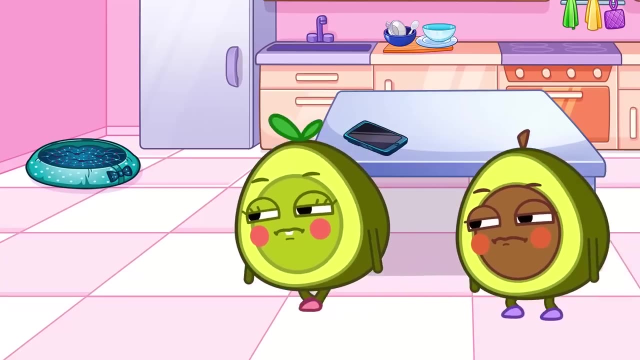 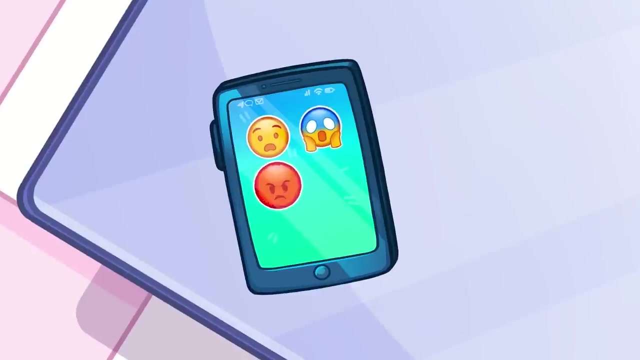 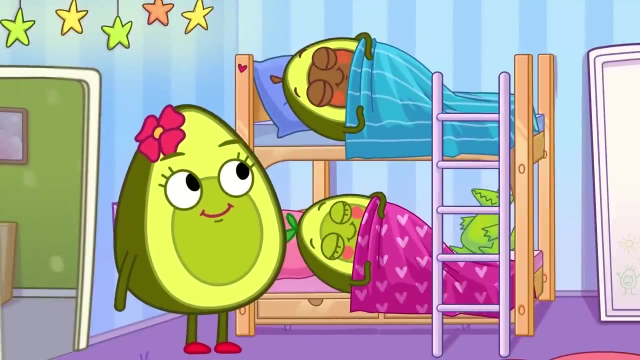 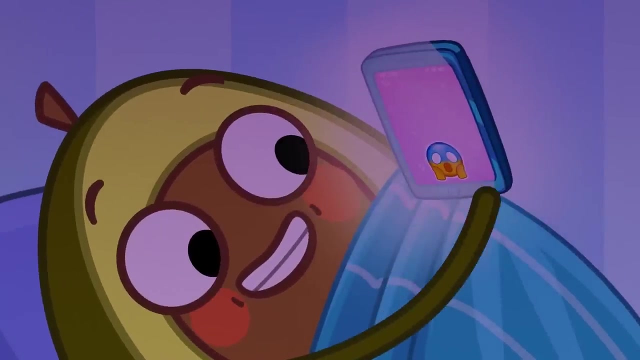 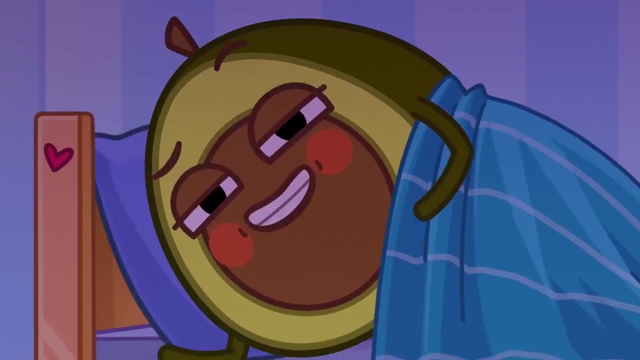 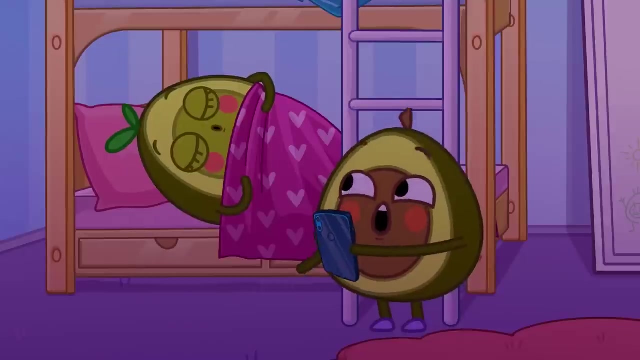 Yay, What a thoughtful gift. Pit and Penny, It's bedtime. What was that? It's a magic emotions app on the phone. Ah, time for sleep Night, Penny. Night Pit. What is Pit up to Joy? 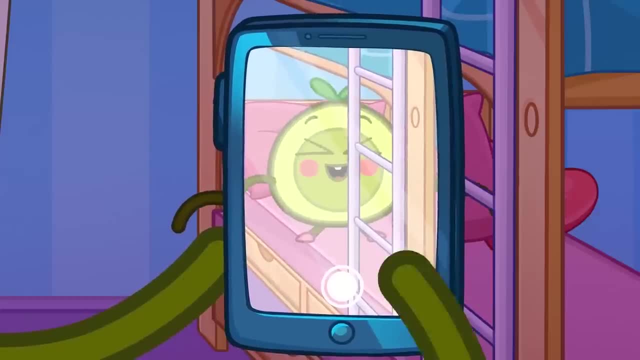 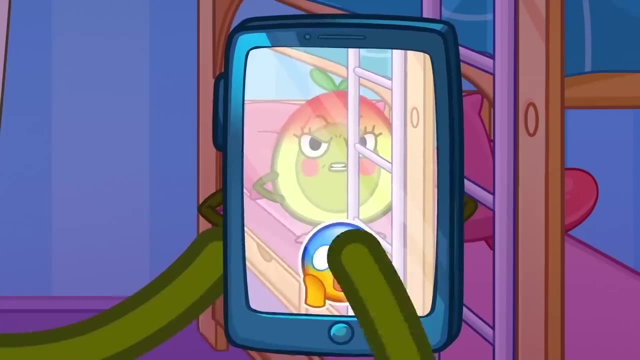 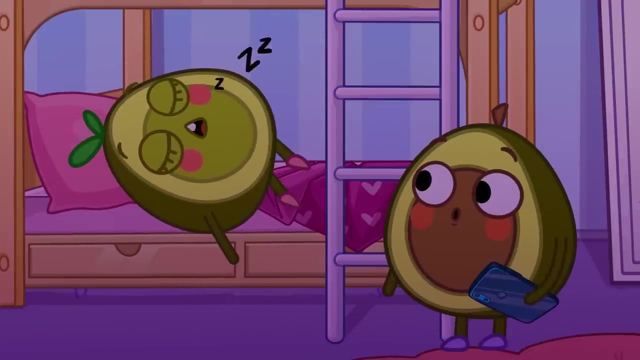 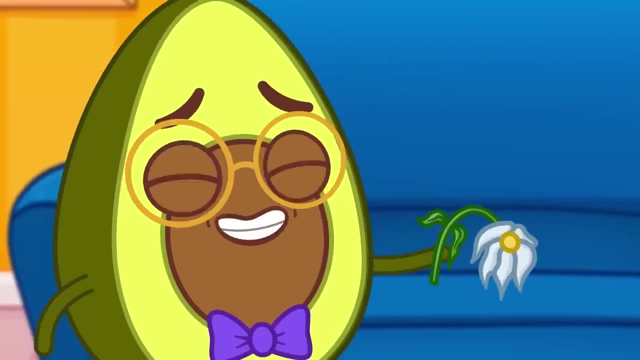 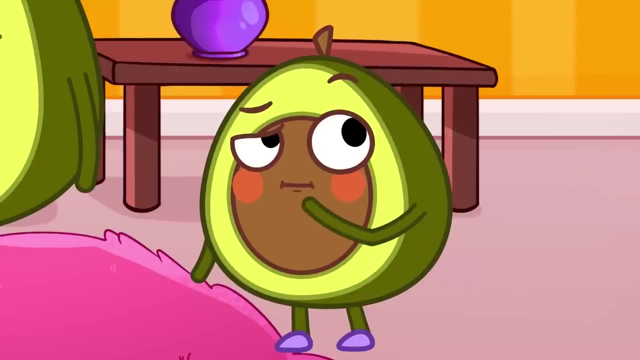 Penny is feeling joyful, But not anymore Sleep. That will put Penny back to sleep. Daddy has a surprise for Mommy. Oh, a wilted flower. What emotion is Pit looking for? Happy, Happy, Happy, Happy, Happy. 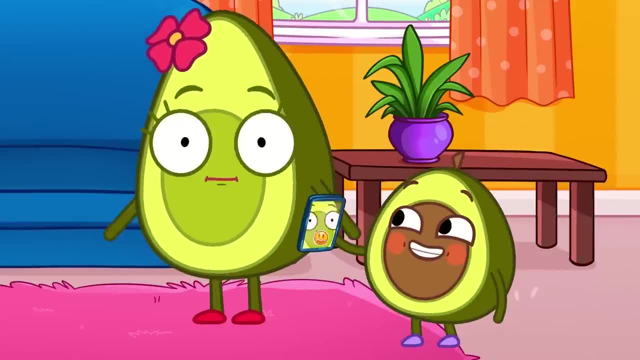 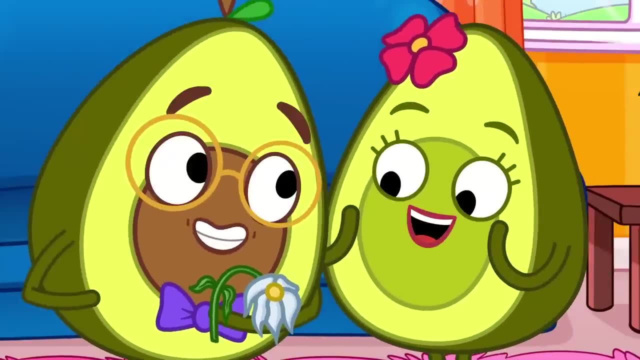 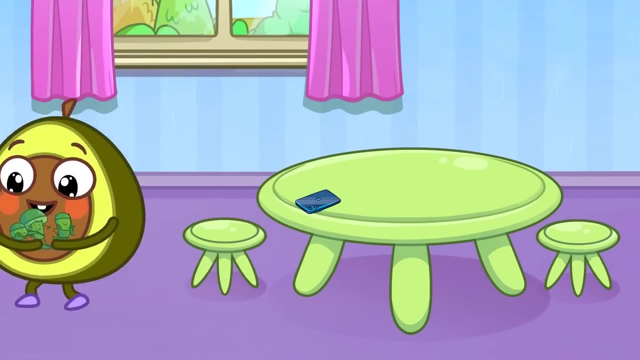 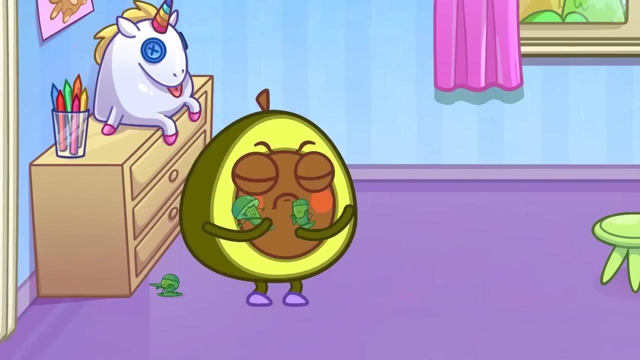 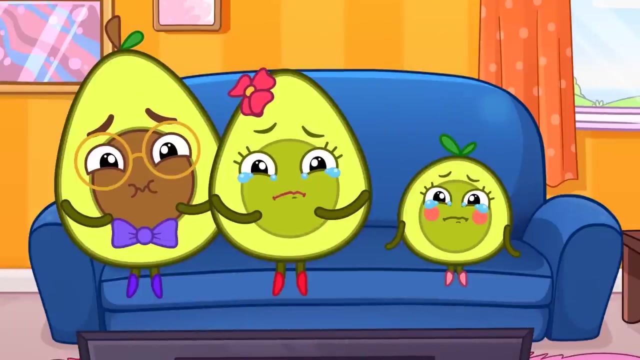 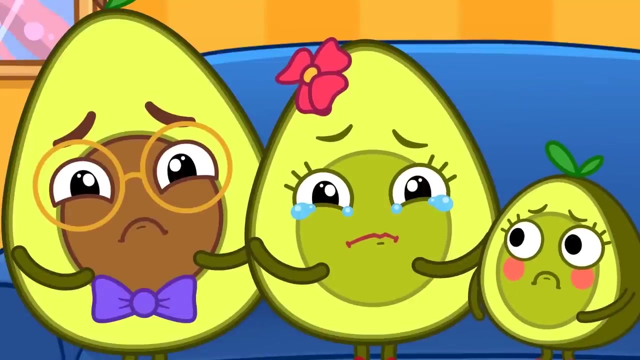 Happy, Happy. Oh Wow, Yes, Mommy and Daddy are happy, Ah ha ha. Quick Penny Change Pit from mad to… Scared. Ah, Ah, Ah Ah. Mommy and Daddy are Dad, But Pit is. 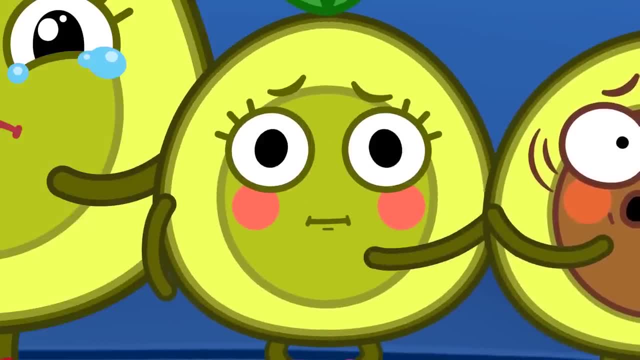 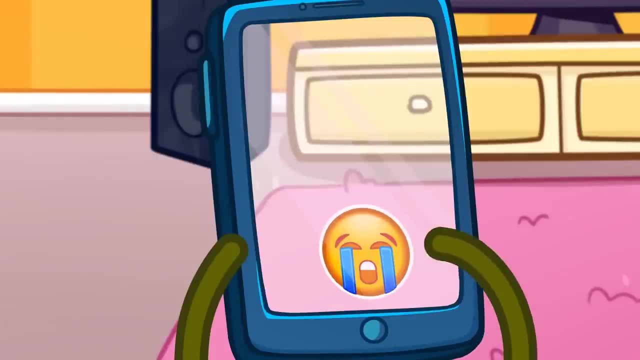 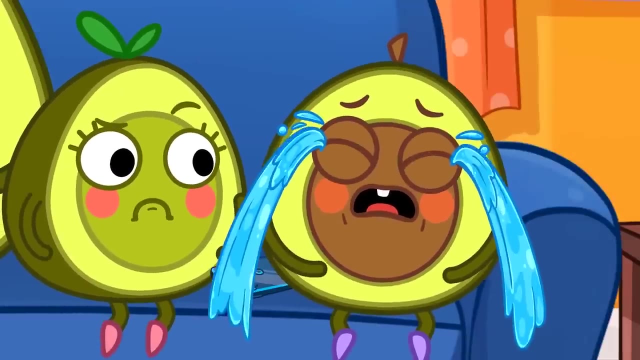 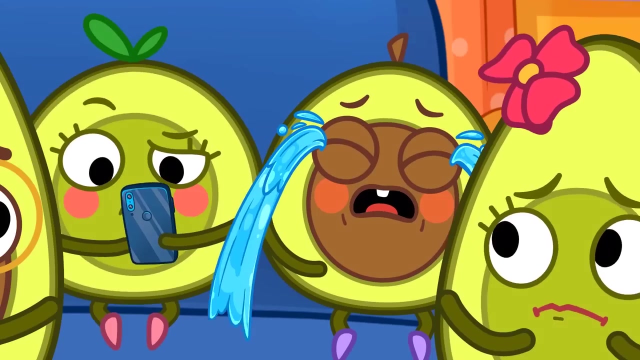 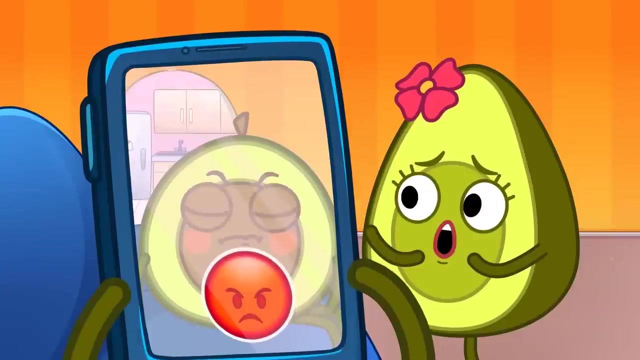 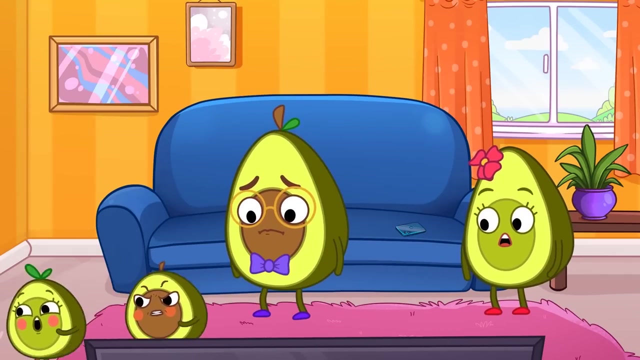 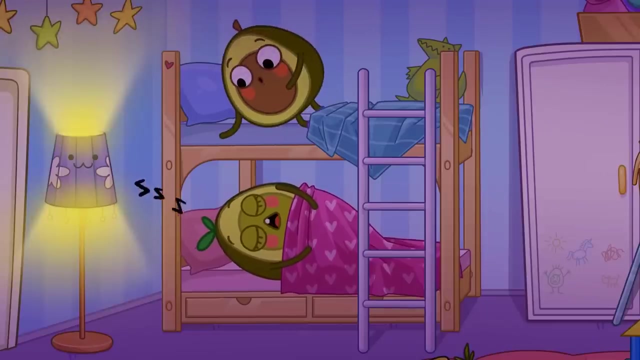 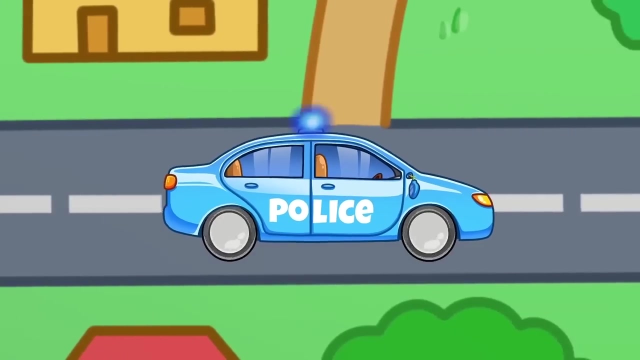 Me, Me. What should Pit be Dad? Oh no, No, not that one. Uh-oh, I'm angry, Angry. Oh no, Phew, It was just a dream. Good night, Pit. Oh, there is an emergency. 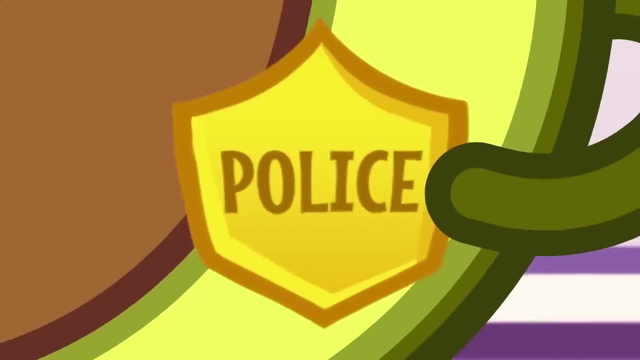 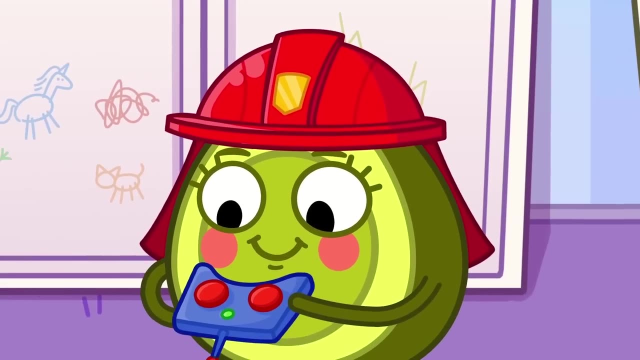 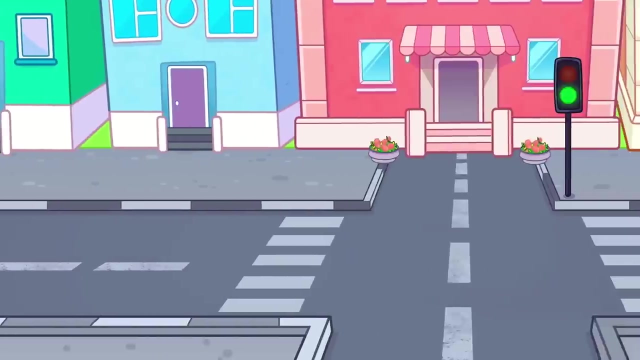 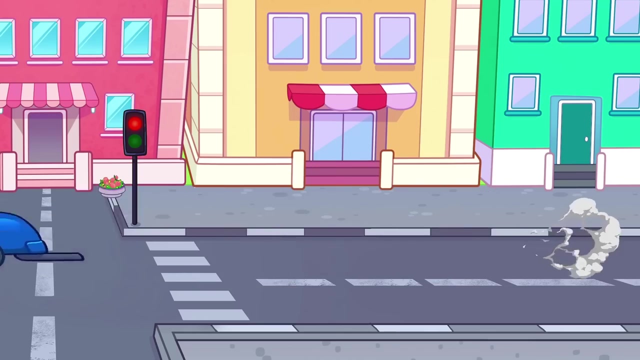 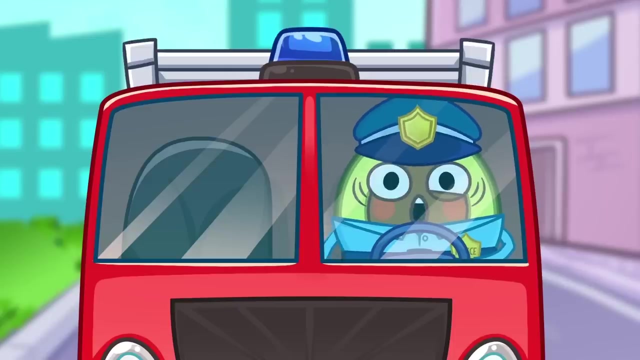 Look out, Pit is a police officer And Penny is a firefighter. But Penny has an idea: It's nice to share toys. The red light means stop. Yeah, This car is being naughty. Pit is in the fire truck. Officer Pit will save the day. 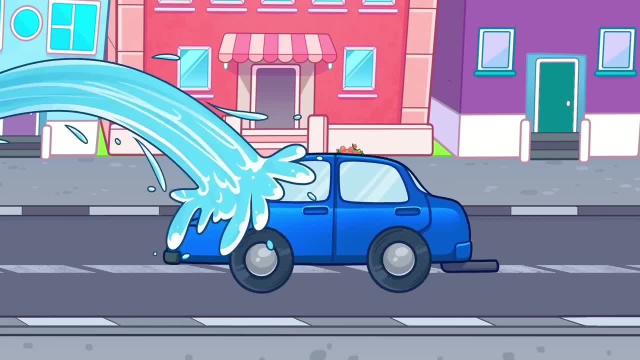 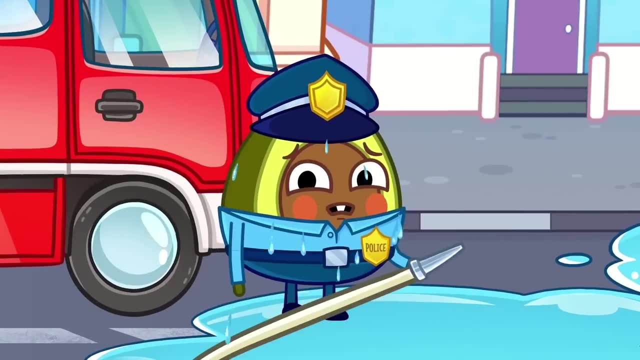 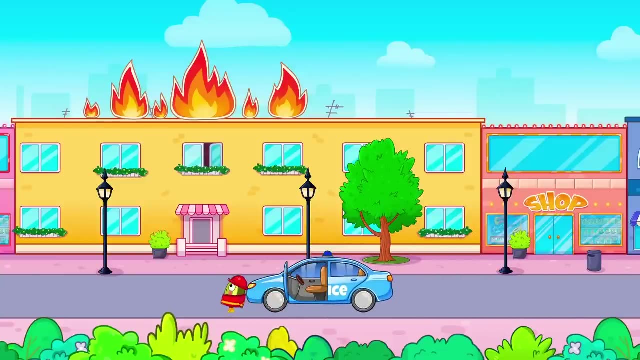 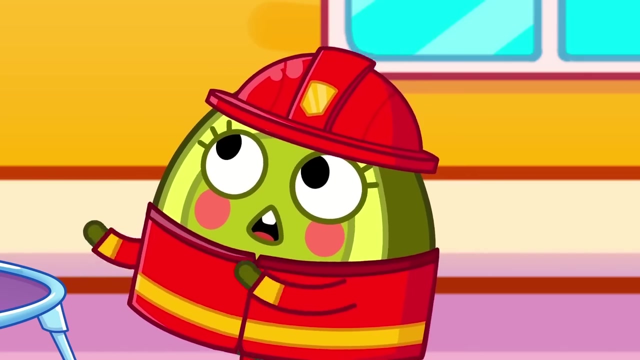 Pit has the fire hose. I'm not sure this will work. The naughty car splashed. Pit Penny is in the police car. Oh no, There's a fire And the kitty is trapped. Jump, kitty Penny is a hero. 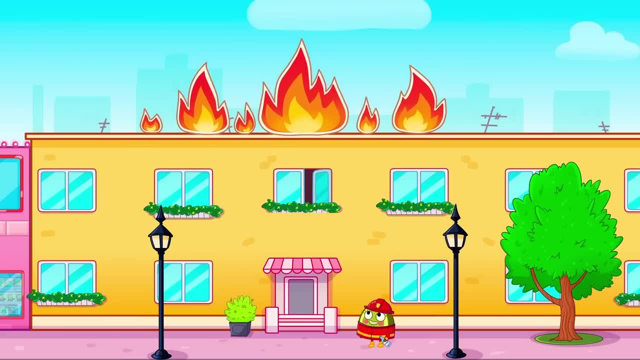 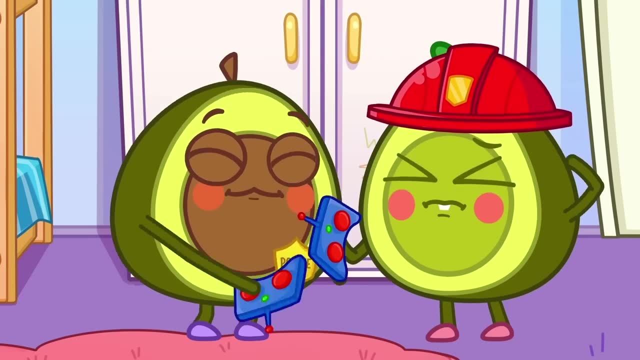 Penny tries to put out the fire, But it doesn't work. Oh, It's a trap. The car is in a bad place. Let's save the kitty. Go, go, go. Why don't you try, Penny? The car is stuck. 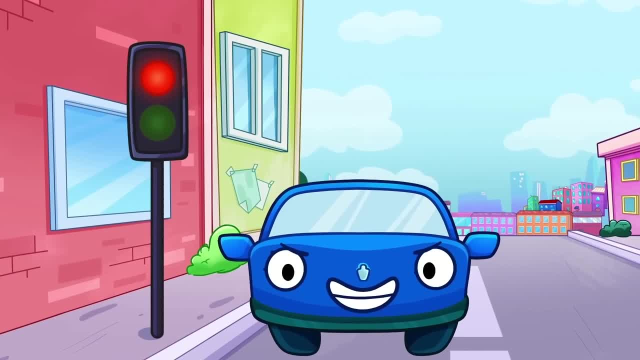 I can't handle it. You can do it, Kitty. One touch and you're safe. It's a good idea. I got a lot of sea slack too. It's so nice. That's what you need. Yeah, a lot. 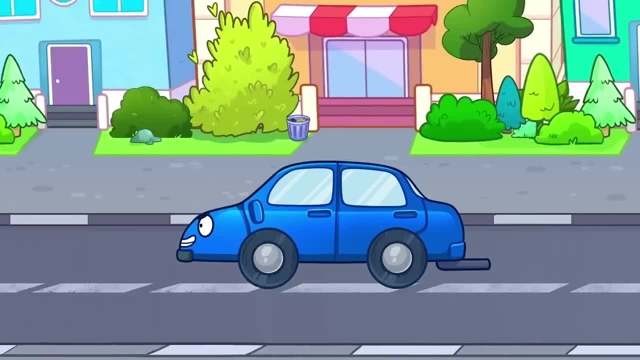 Phew, You're so lucky, Penny. It's not scary to be a little bit crazy. I'm proud of you. Tell me about your big sister, Penny. Oh, I heard you. Of course, I'm going to give you a big kiss. 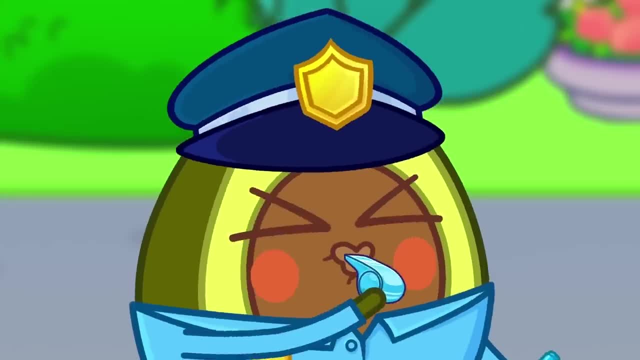 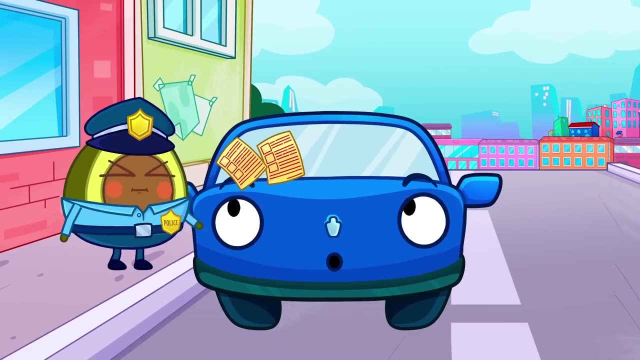 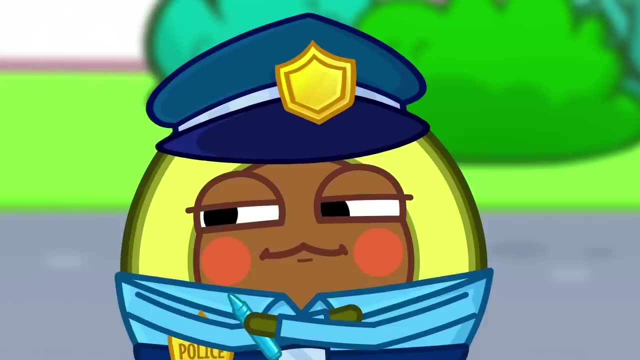 It's not funny. She loves to dance. Put your phone down. Put your phone down. Put your phone down And the car can't park here. The car is angry. Good job, Pit Penny has the fire hose this time. 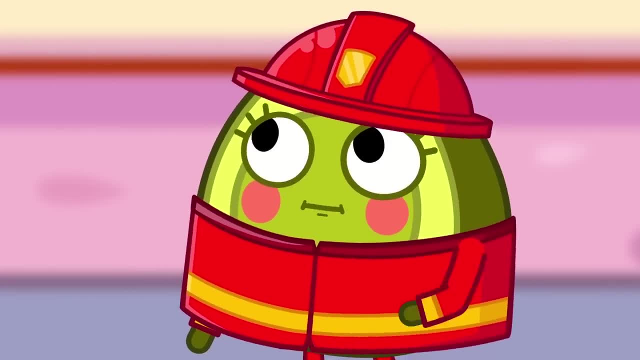 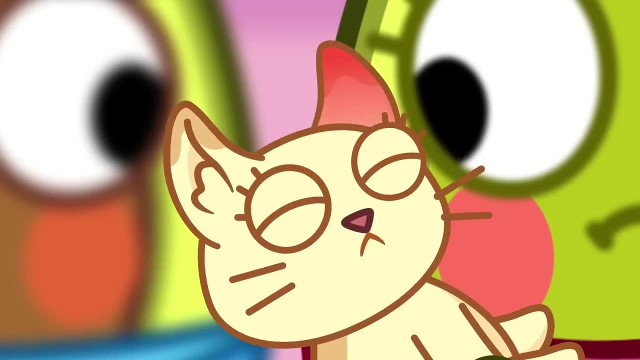 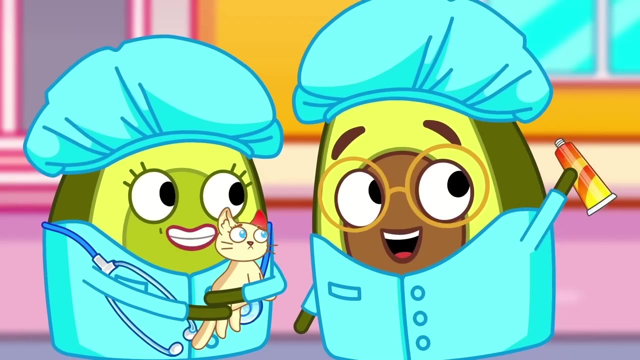 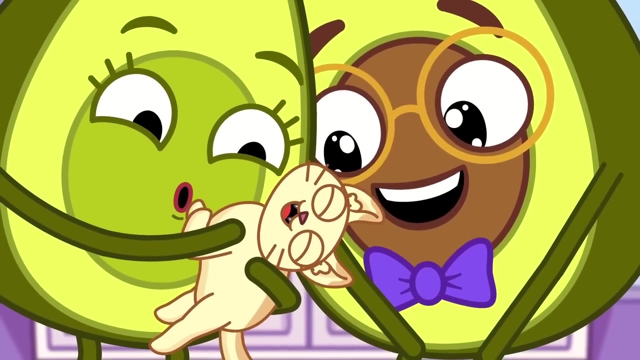 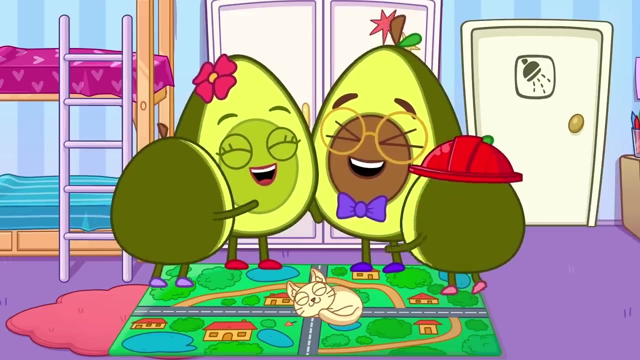 Look, The fire is going out. The kitty has a sore ear, Don't worry, Mommy and Daddy are here. Daddy has special cream to help the kitty. Aw, everyone gets kitty hugs. Kitty is tired after all that excitement. What a great adventure. 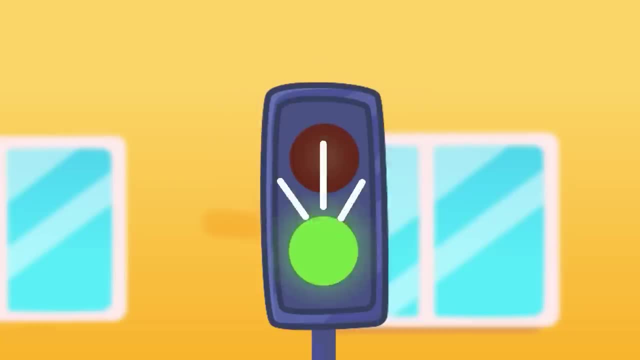 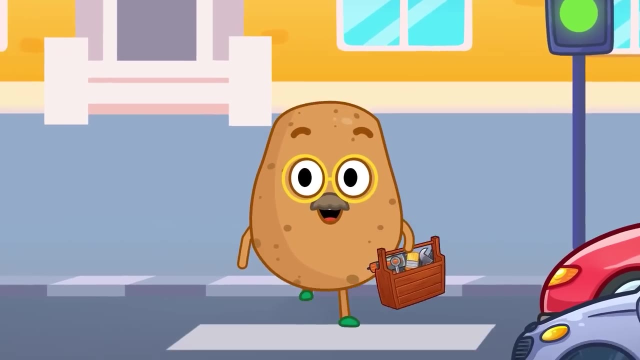 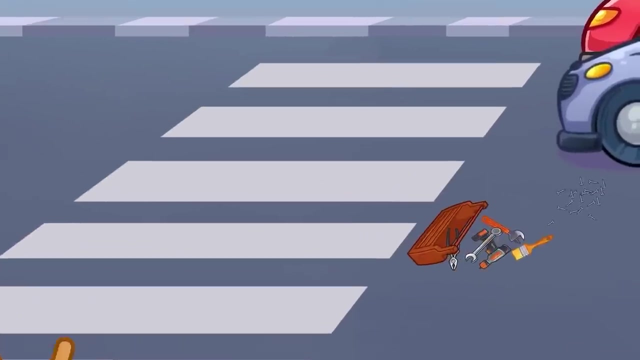 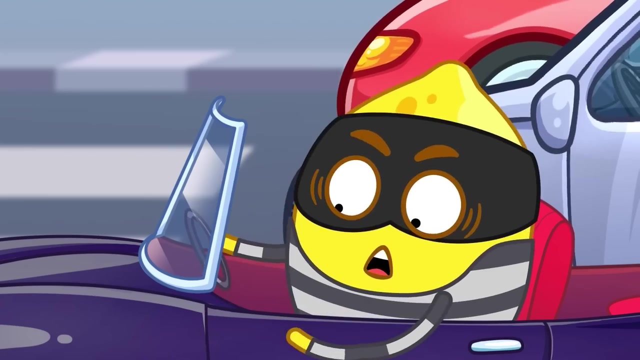 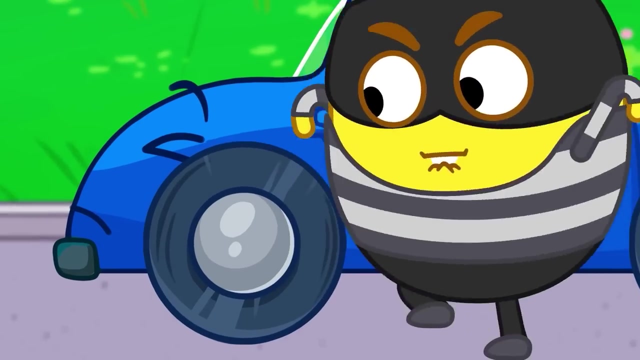 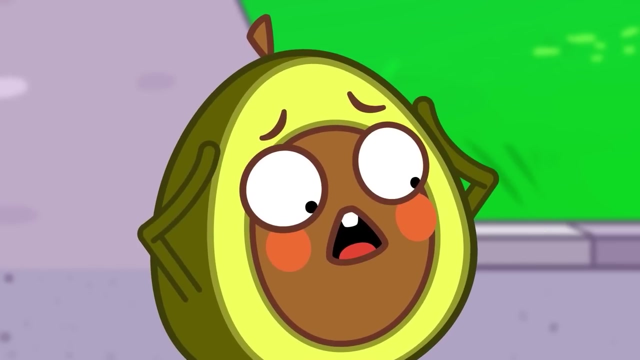 What is Mr Lemon up to today? The green light means Potato can go. Watch out for Mr Lemon. Now Mr Lemon has a flat tire. Oh no, He's stealing a wheel from Pit's car. Look, Pit, Something's missing. 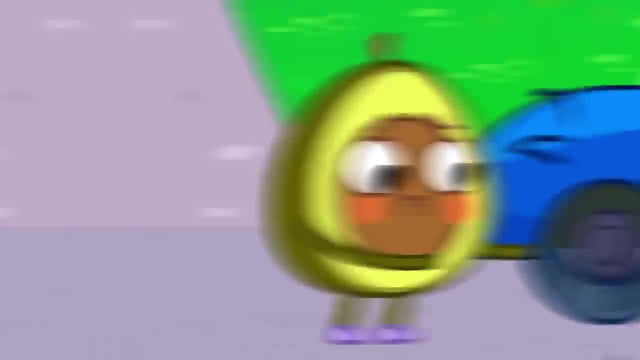 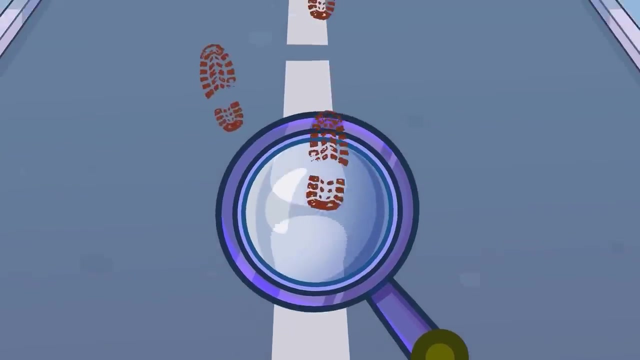 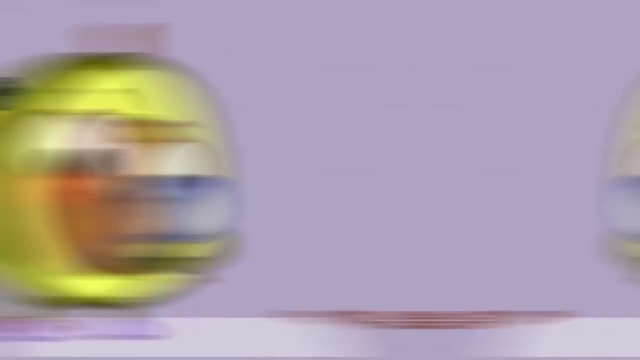 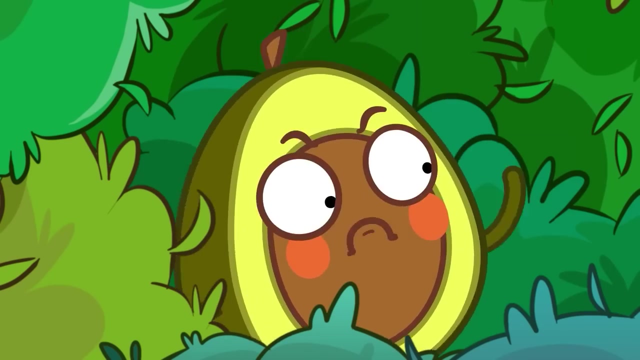 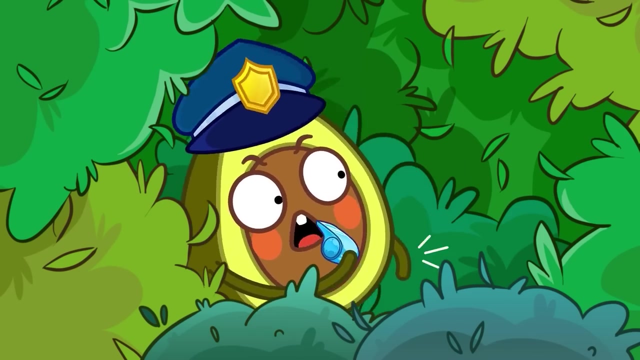 Oh no, Where is my wheel? Let's look for clues. It's a footprint. Follow them and see where they go. Oh, It's Mr Lemon and the missing wheel. Time to catch the criminal. You better stop, Mr Lemon. 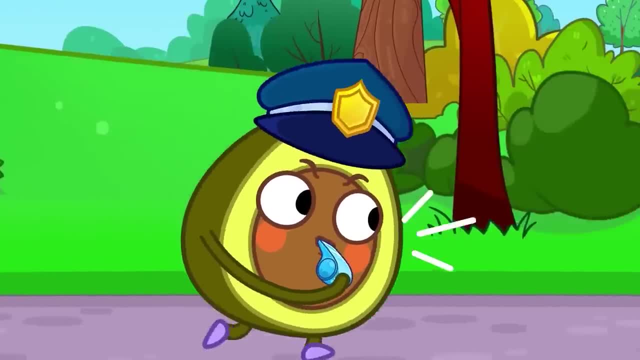 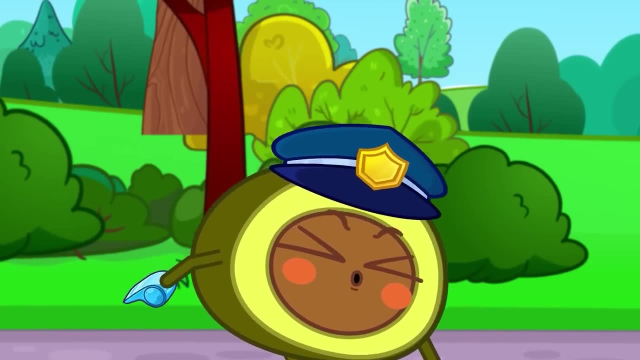 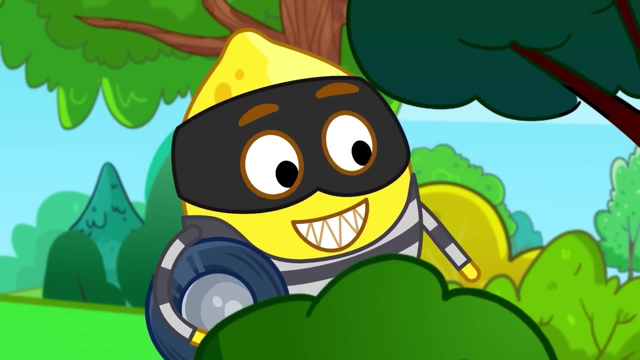 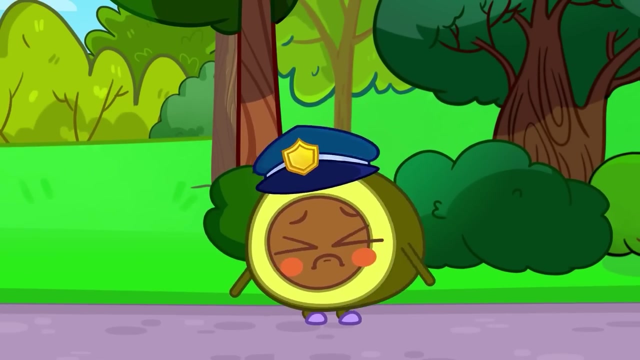 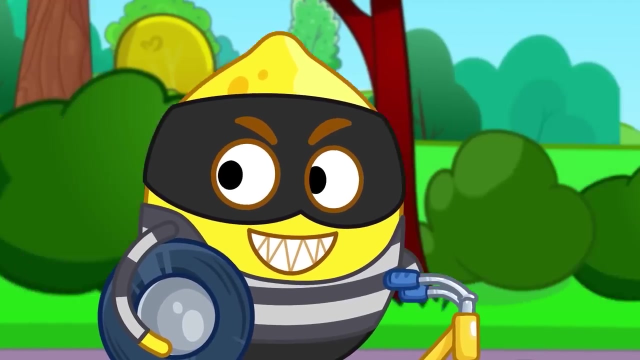 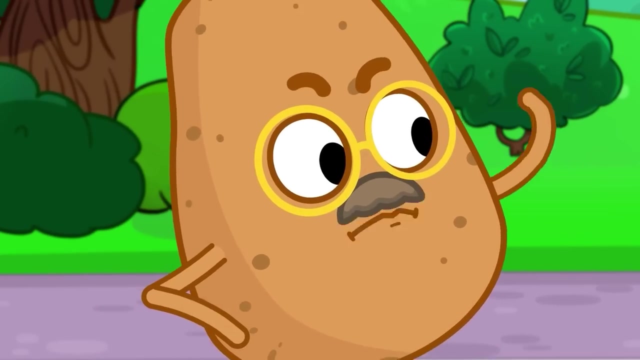 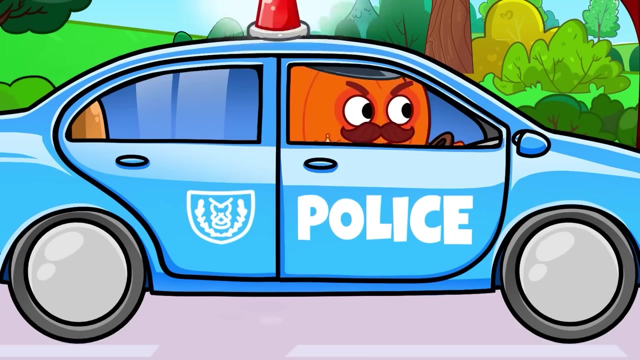 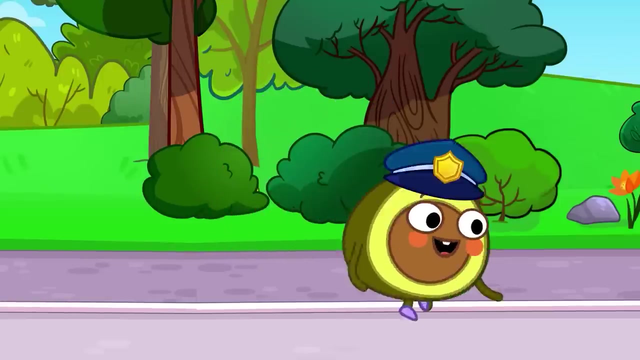 Pit is on the case. Mr Lemon is too fast. Where did he go? Mr Lemon stole a bike. It belongs to Potato. Give me back my bike. Huh, Officer. Pumpkin Pit needs your help. Can Pit and Pumpkin catch the thief? 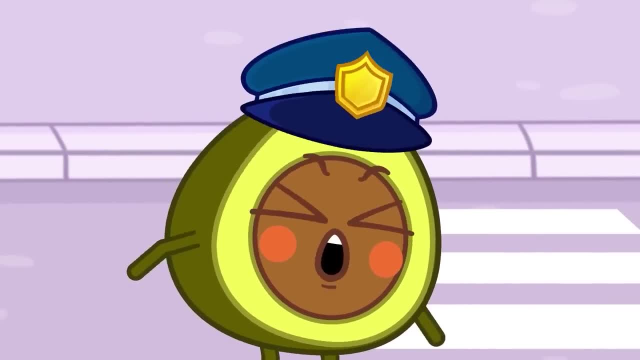 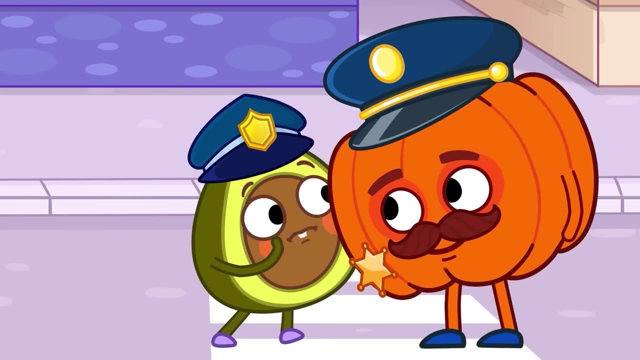 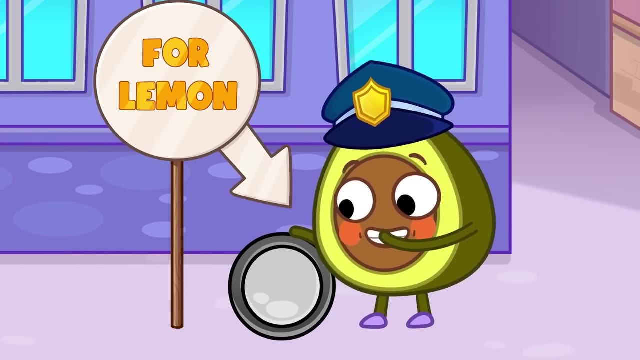 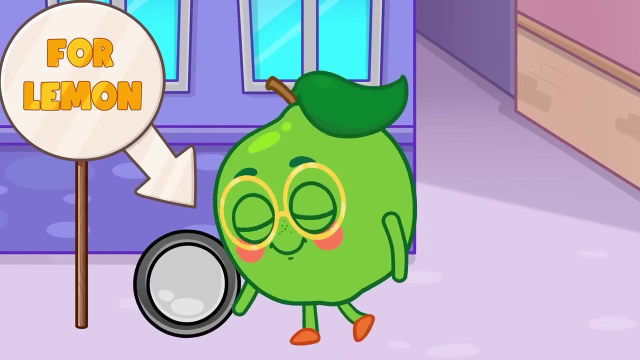 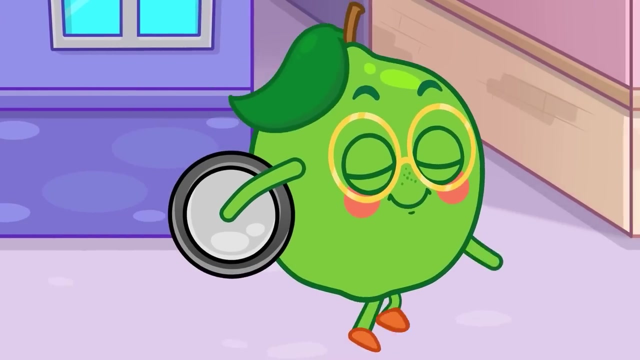 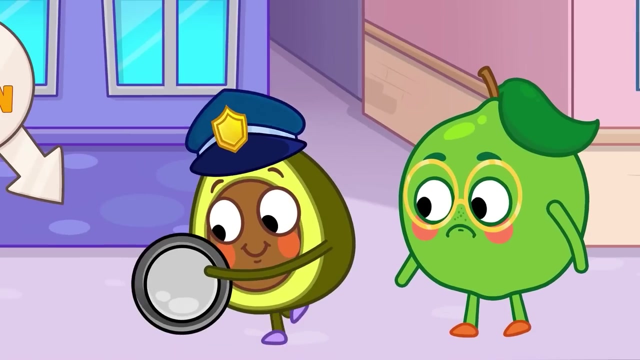 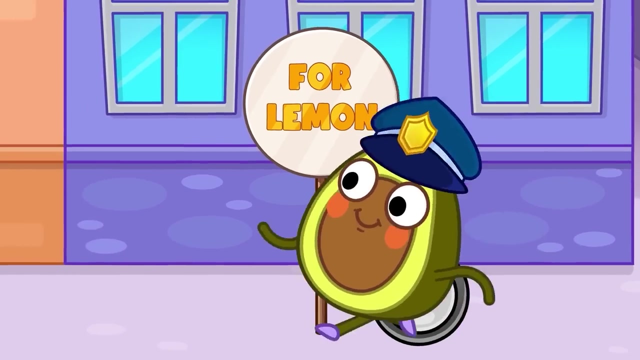 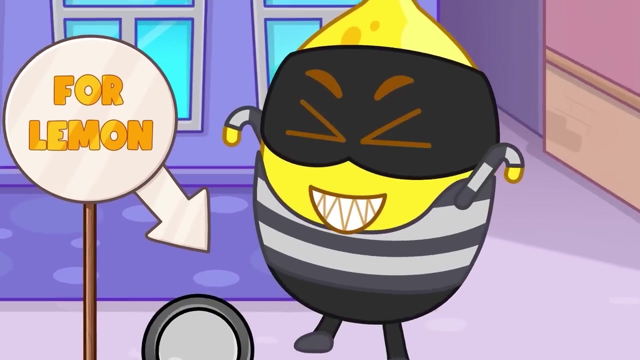 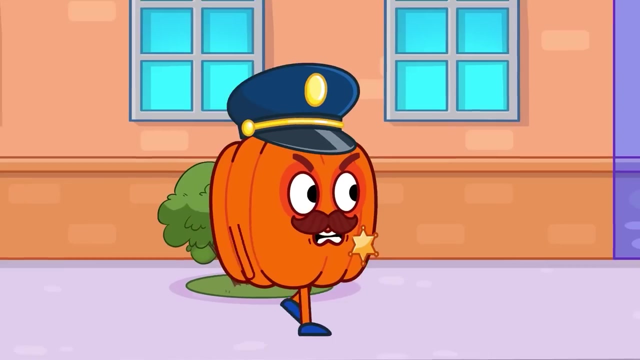 He got away again. But Pit has an idea: He set a trap for Mr Lemon. Here comes Lime. No, Lime, That's not yours. Here comes Mr Lemon. Hey, You are under arrest. Well done, officer. 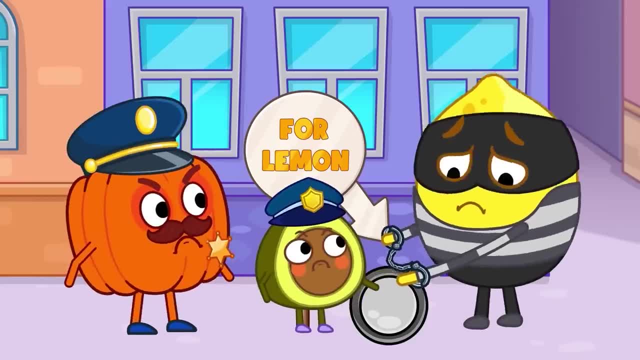 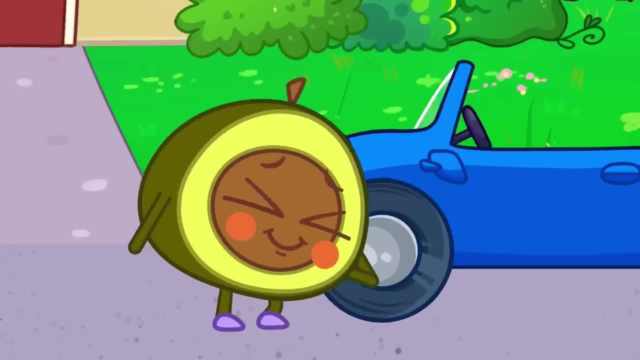 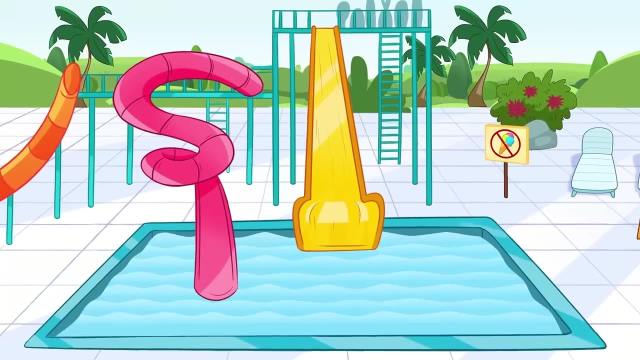 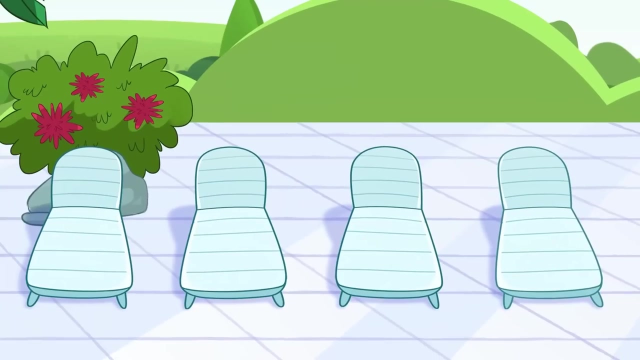 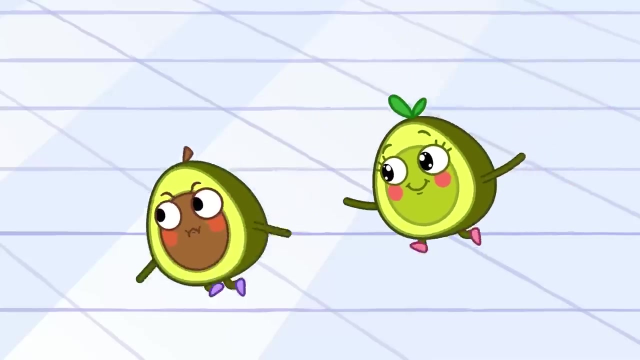 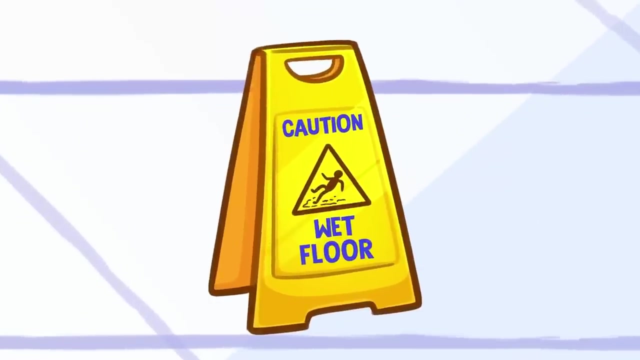 You must stop at the red traffic light. Yay, Pit's car is back to normal Time to solve more crimes. Pit and Penny are still at the pool And Penny is super excited. The floor is wet and slippery. No running. 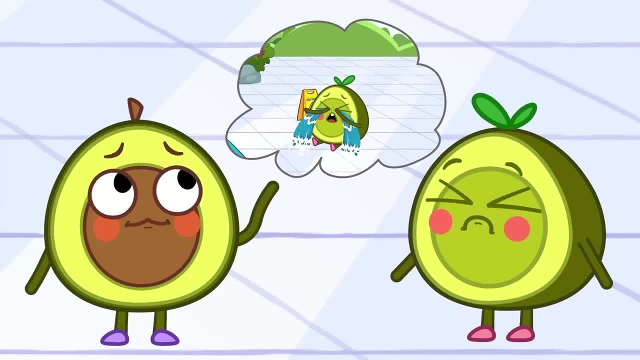 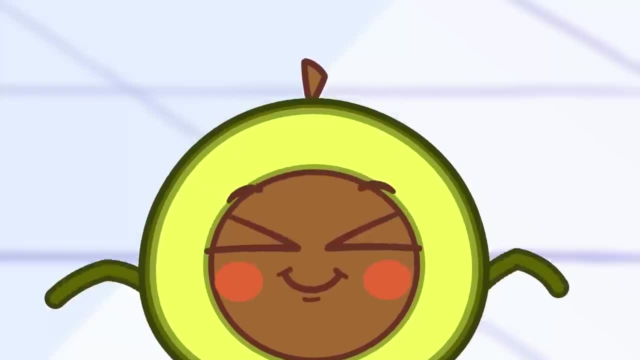 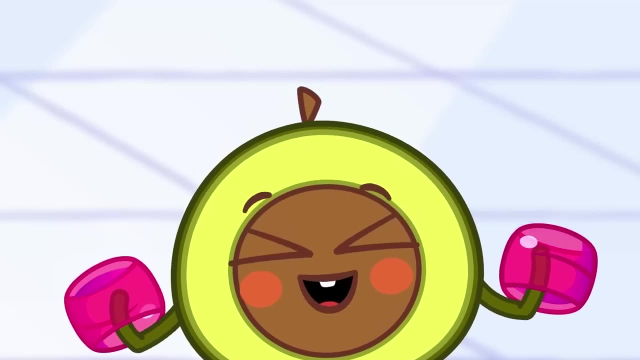 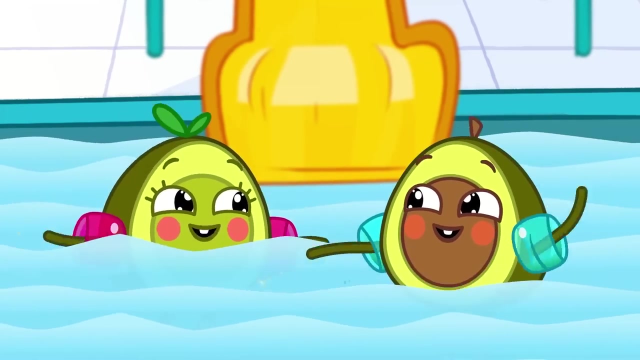 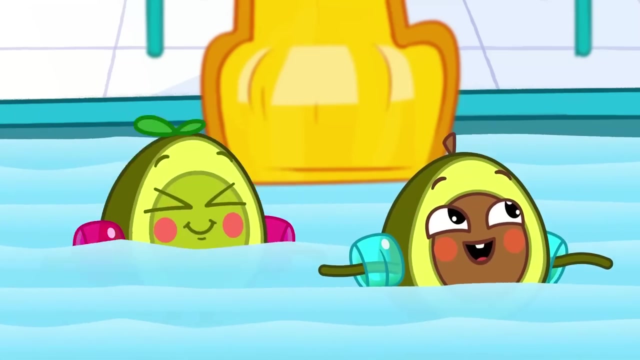 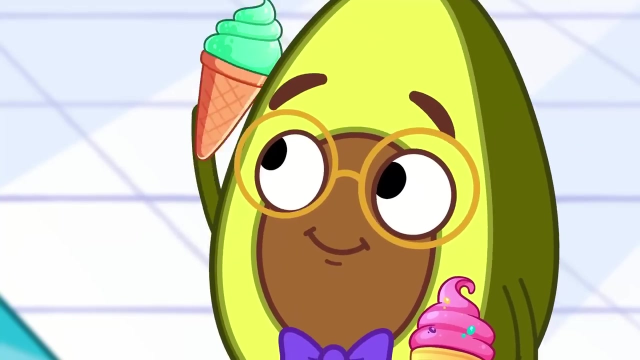 You could get hurt. That's better, Penny. Wait, Penny, Don't forget your floaties. Pit Penny, Ice cream Yum. You can't eat ice cream in the pool. No, No, No, No, No. 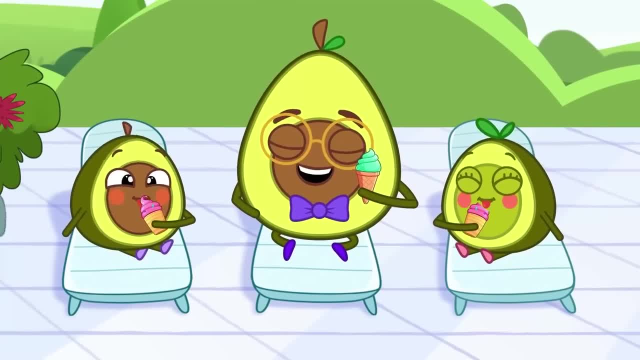 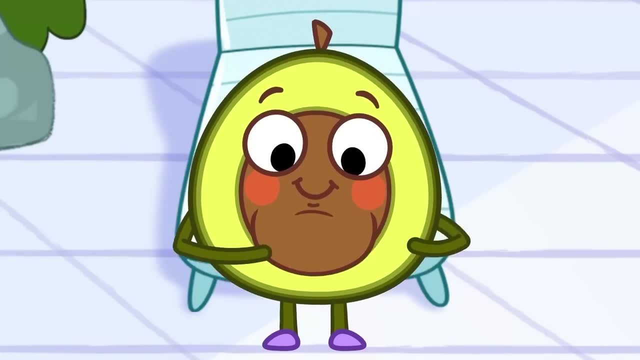 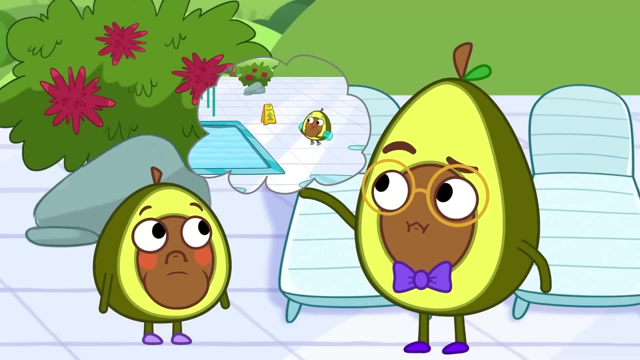 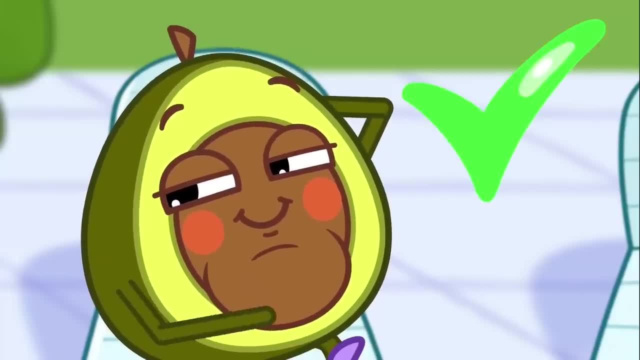 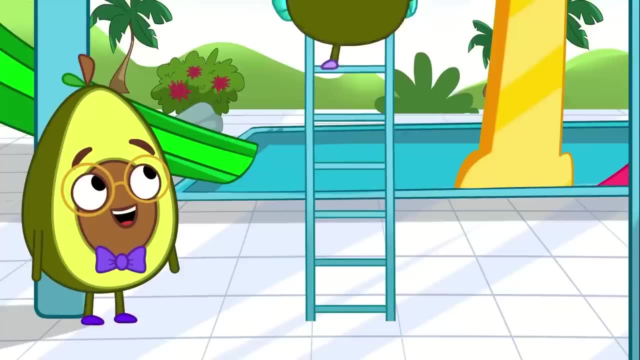 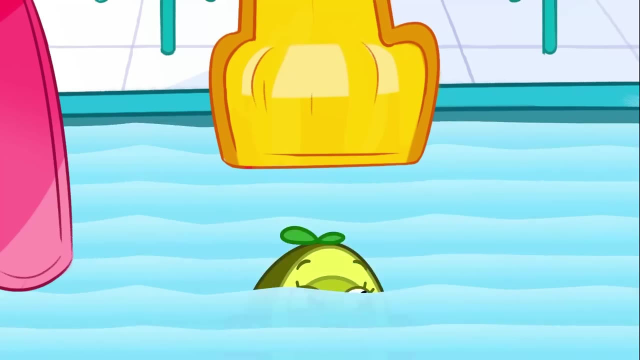 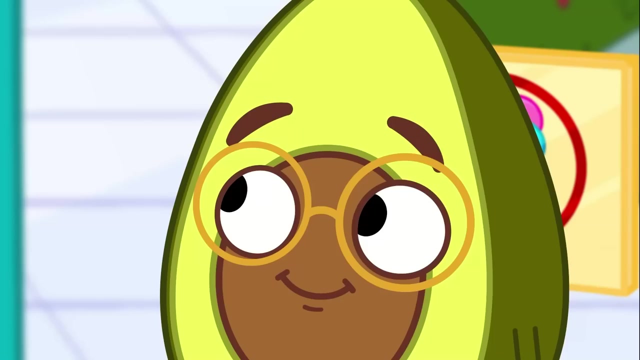 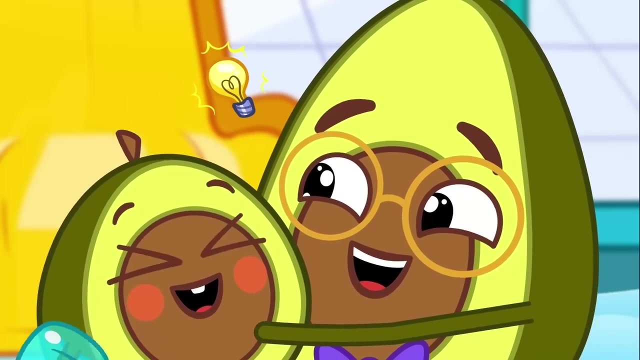 This way, Pit can plan his next adventure. Pit and Penny want to try the big water slide next. It's Penny's turn first, And now it's Pit's turn. Watch out, Penny. Phew, that was close. Maybe going down together will be safer. 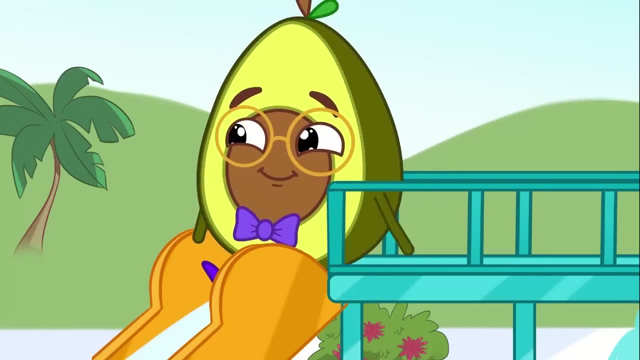 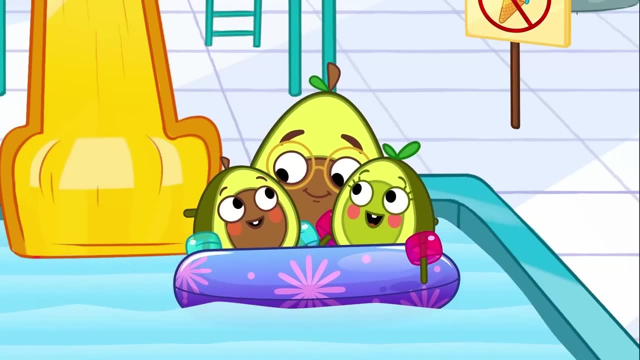 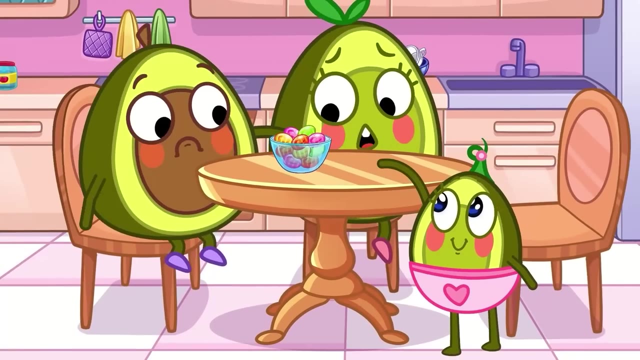 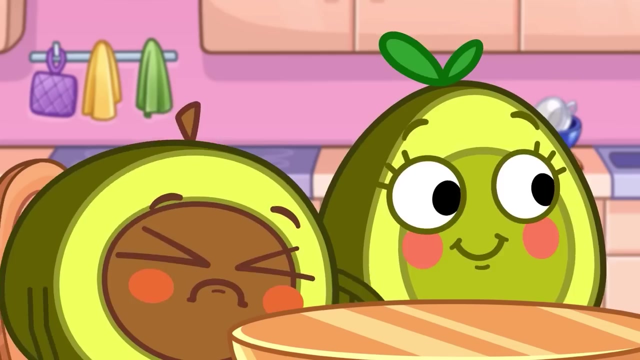 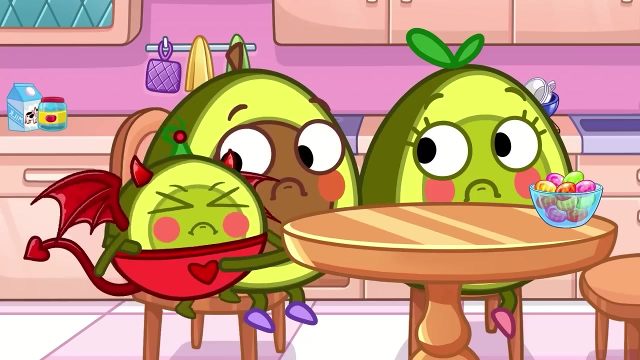 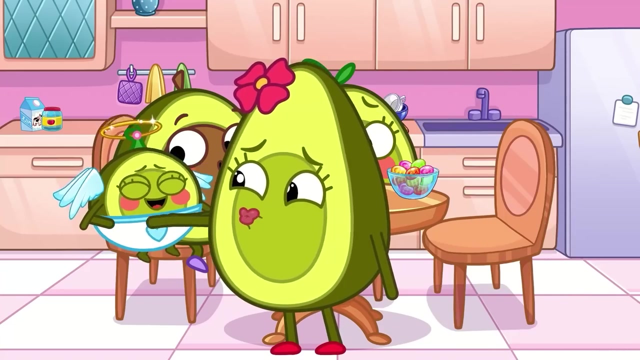 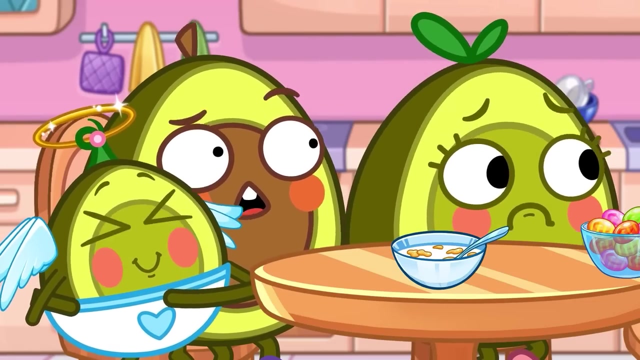 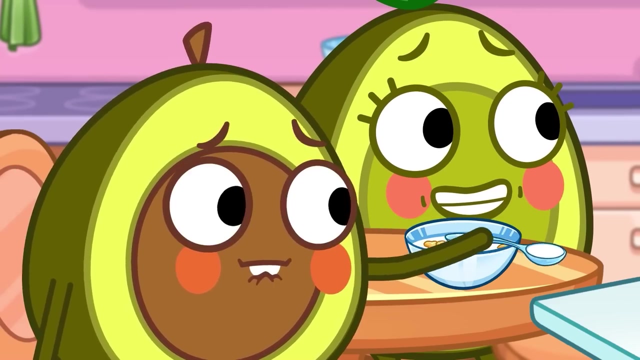 Where's Daddy? Have fun and play safe. Uh-oh, Baby wants some candy, But candy isn't good for Babies. Here comes Mommy Now. Baby won't behave herself. Can you fit your little sister? Uh-oh… Okay, Pit time to feed Baby. 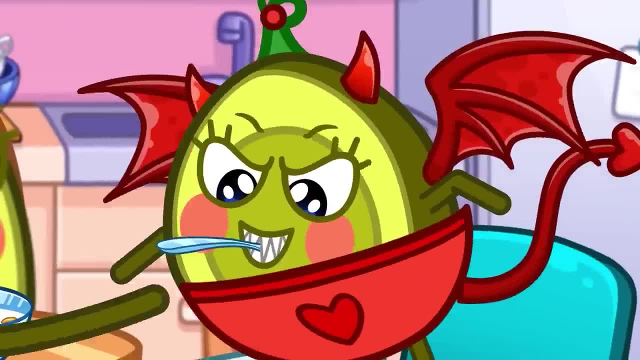 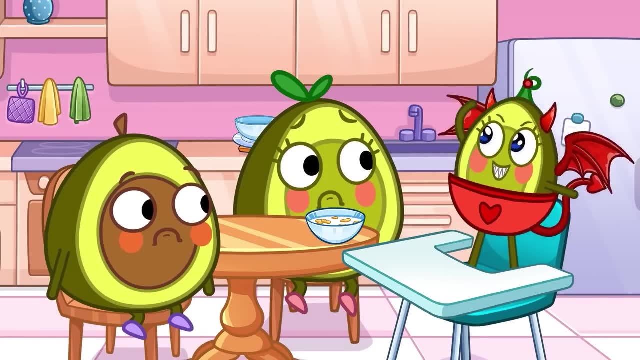 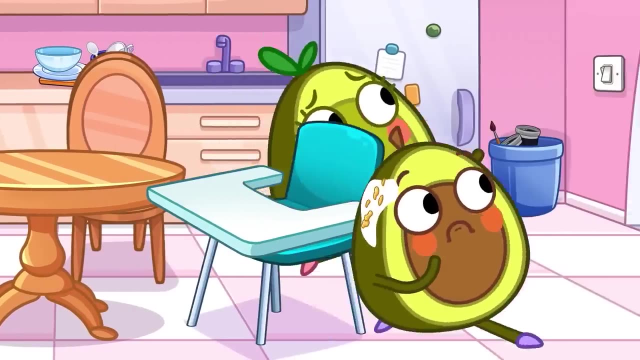 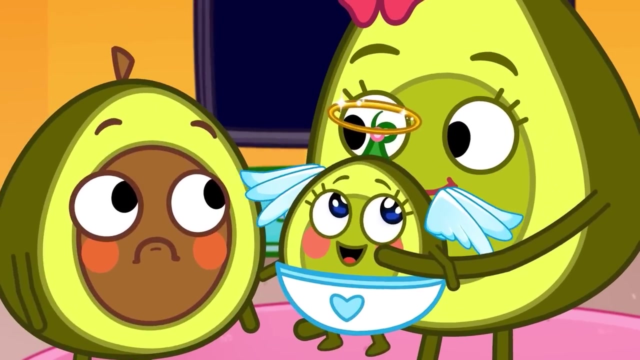 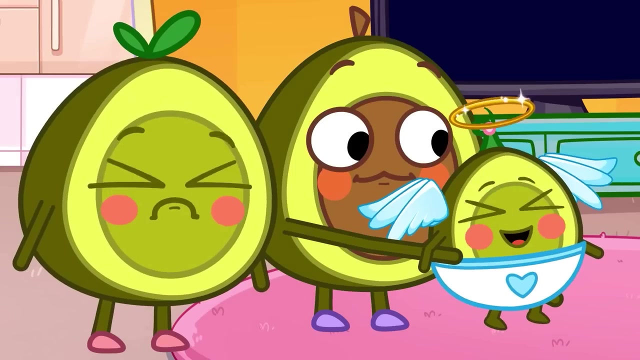 But Baby's being naughty again. Baby, that's not very nice. Whoooa, Baby is being sweet again. Look after your little sister while I clean up. Oh, Baby made a little mess. I'm sorry, baby, I'm so sorry. 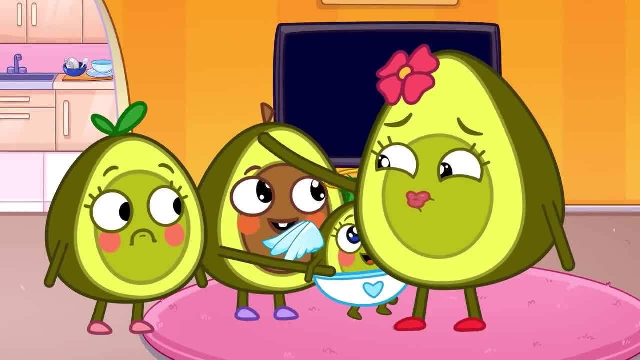 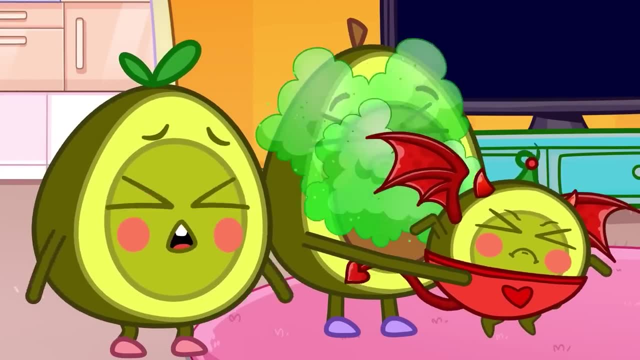 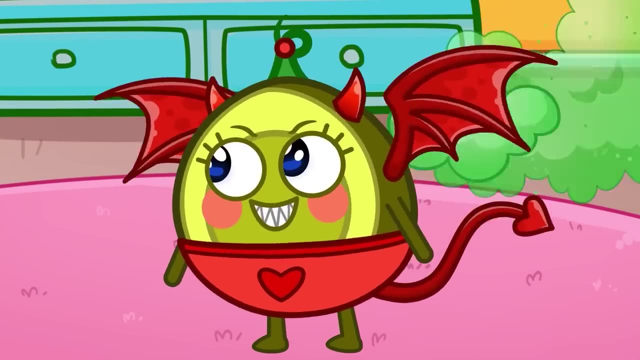 Baby, let's just go home. Okay, See you on the next adventure. Bye, See you on the next adventure, Bye, Bye, Bye, Bye, Bye. Ooh, baby made us stinky And she won't stop. 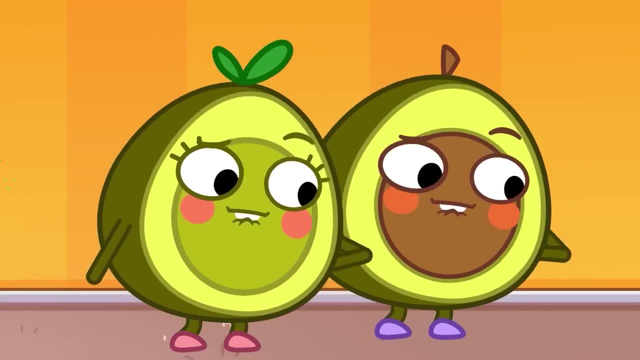 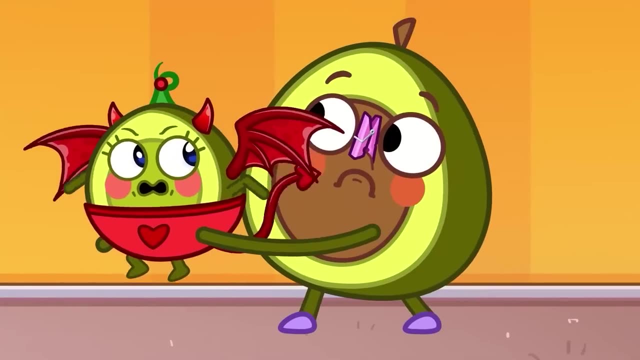 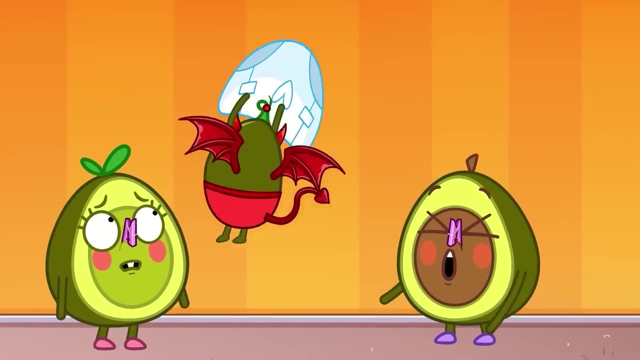 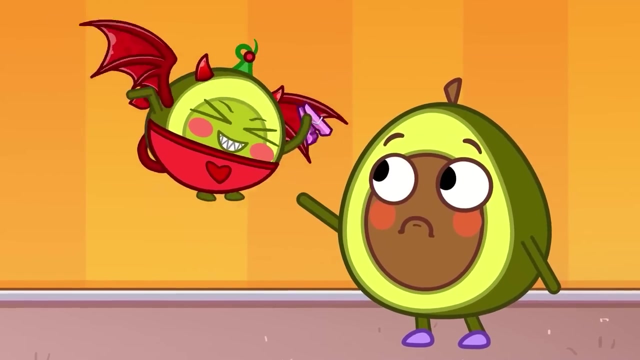 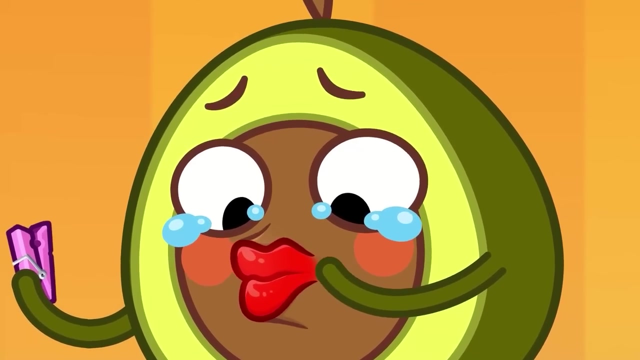 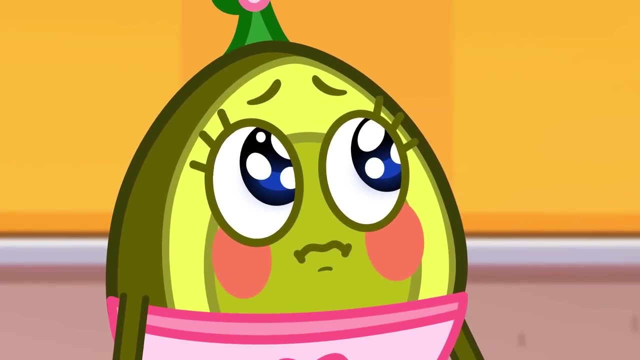 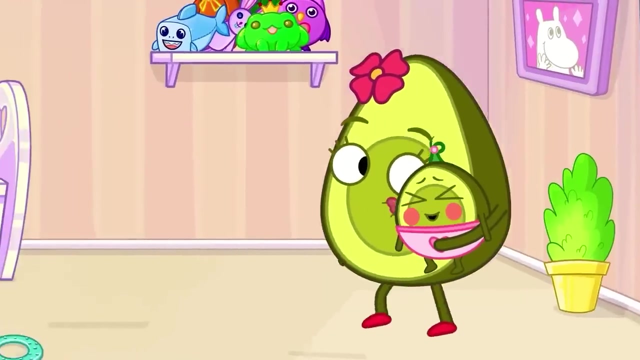 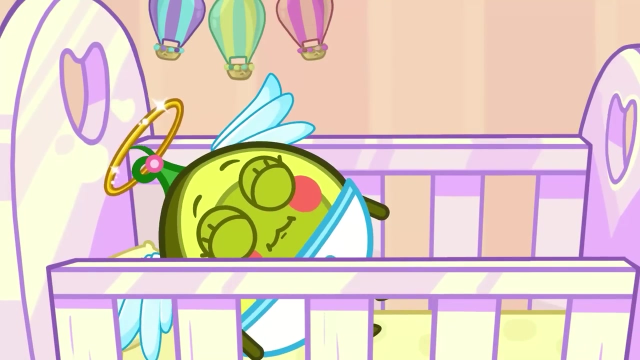 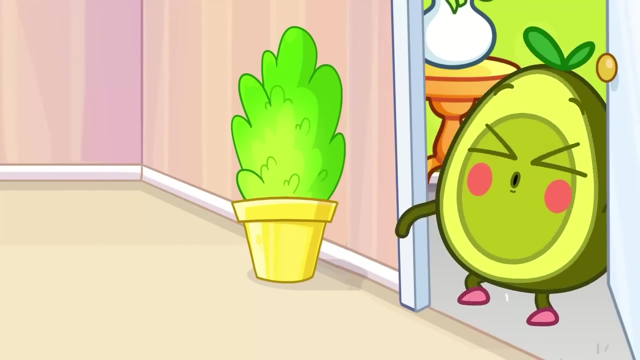 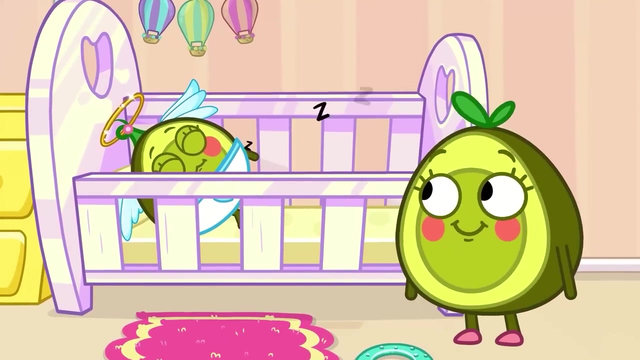 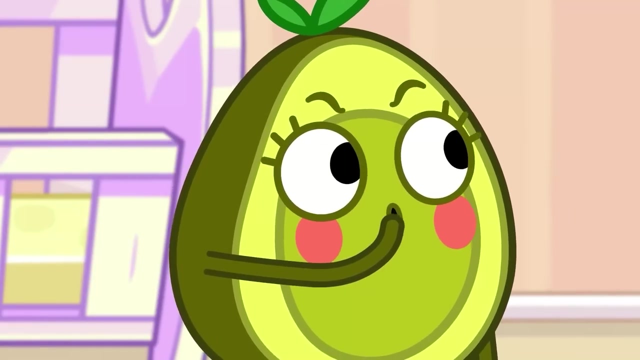 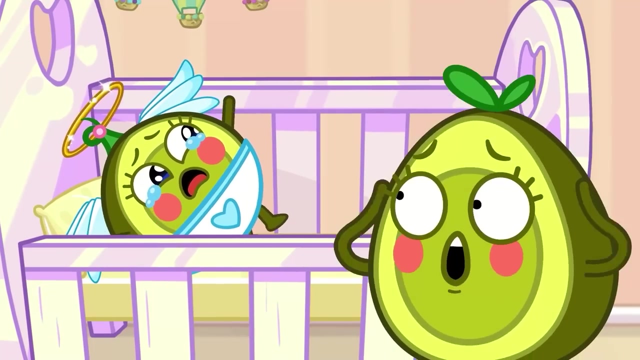 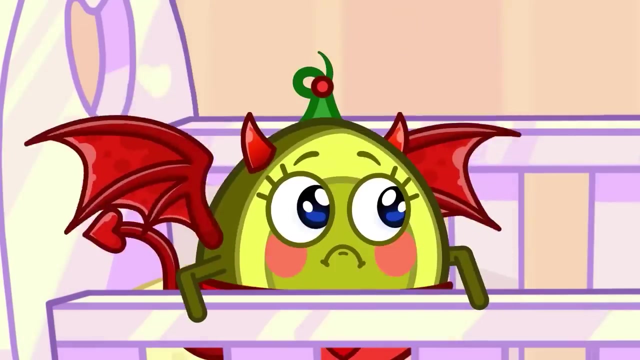 Pit Penny, Cover your nose. Time to change baby's diaper. Poor Penny, Poor Pit. Maybe mommy can help. It's time for baby's nap. Shh, Baby's sleeping. Watch out, Pit Shh, Naughty again. 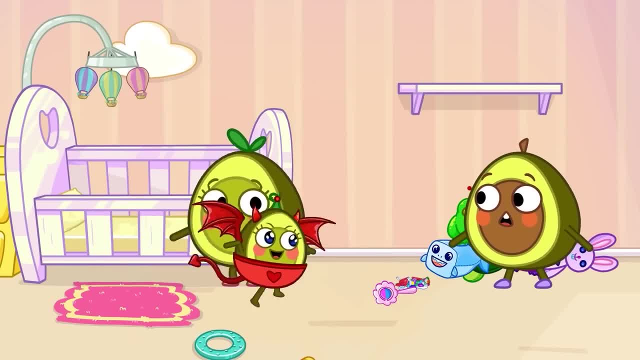 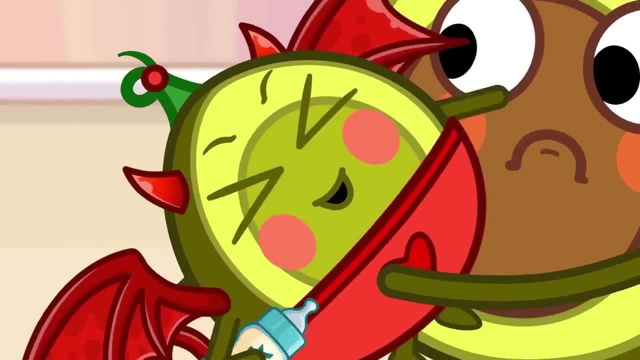 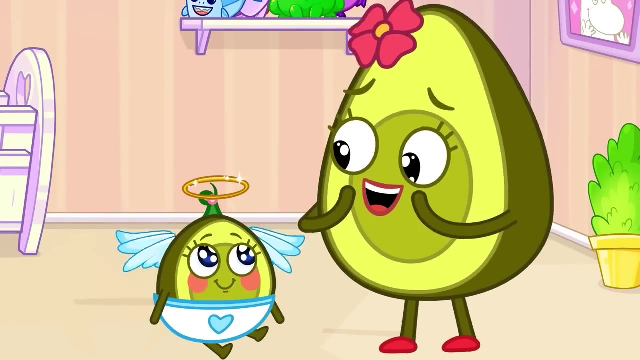 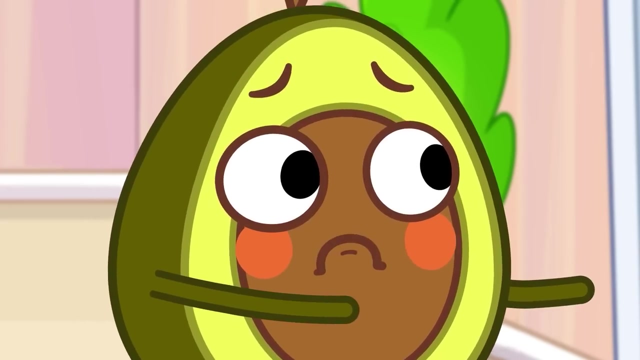 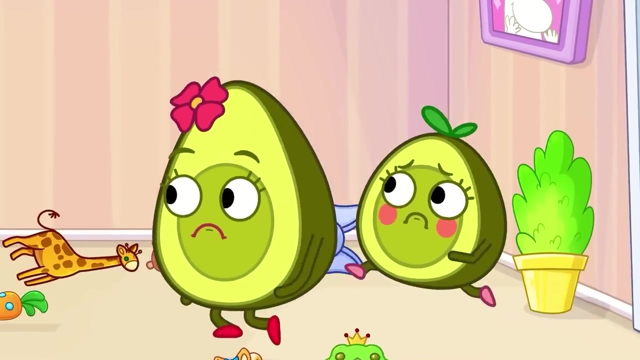 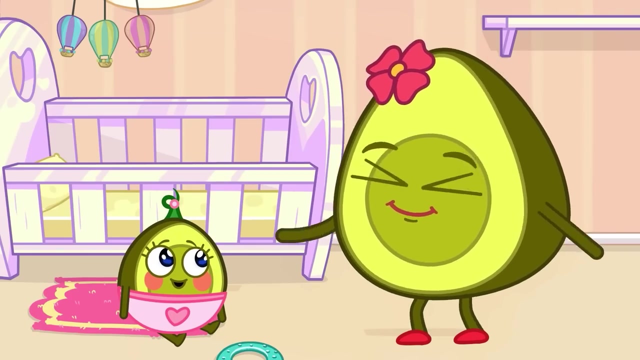 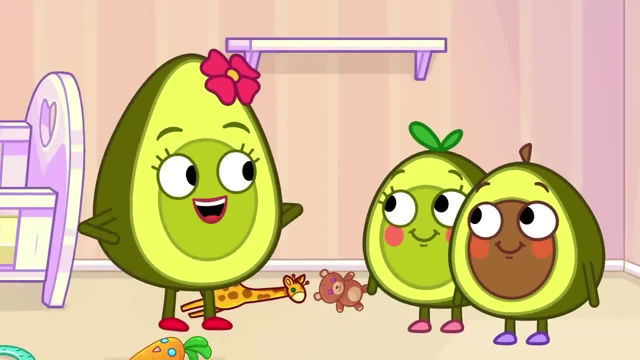 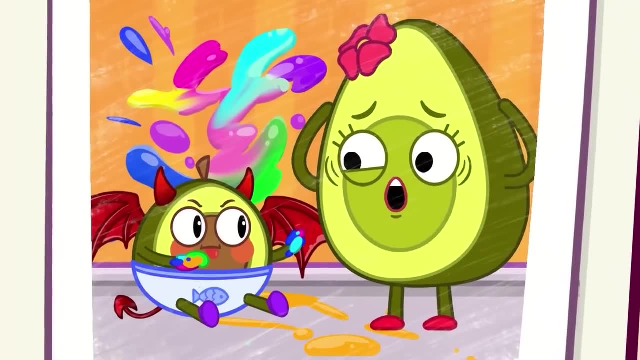 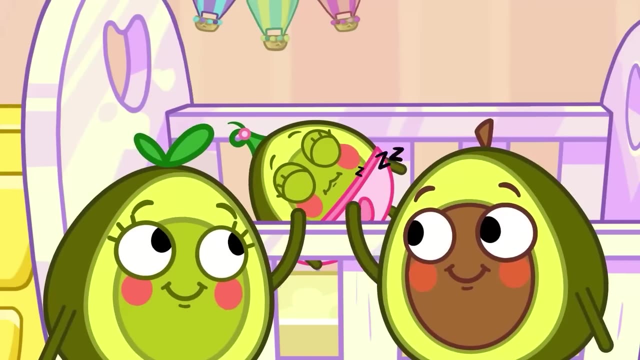 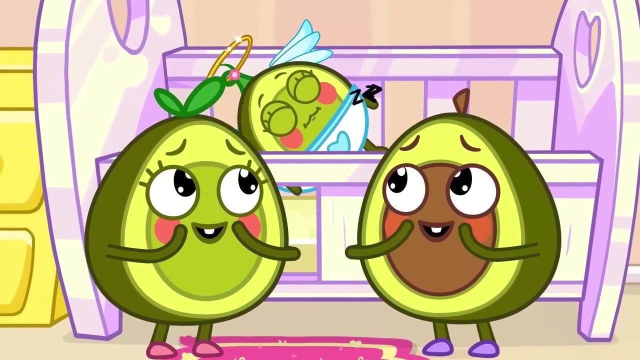 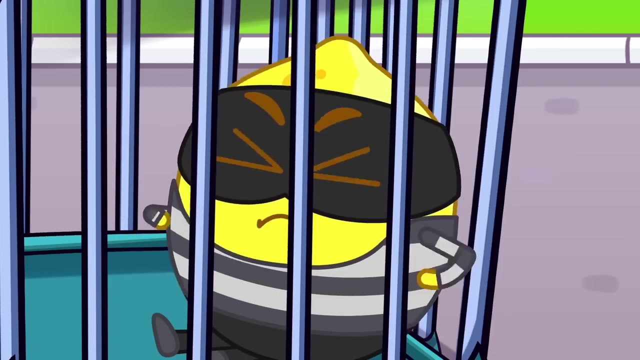 Kids can be naughty sometimes, but that's okay. Even Penny and Pit were naughty as babies. Thank you for your patience. Aw, Baby's, a sweet little angel again. Oh no, Mr Lemon is trying to steal the baby elephant. The baby elephant ran away to hide. 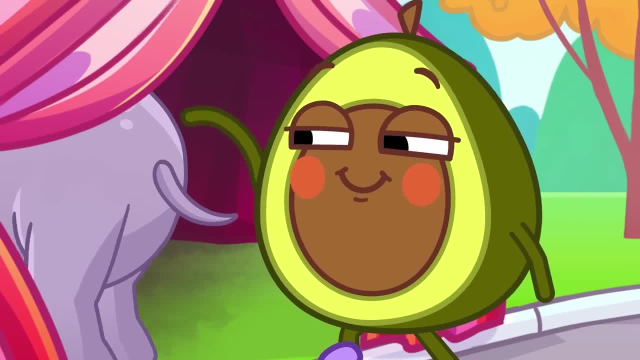 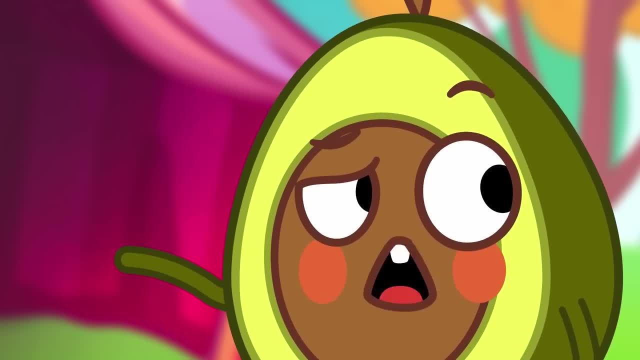 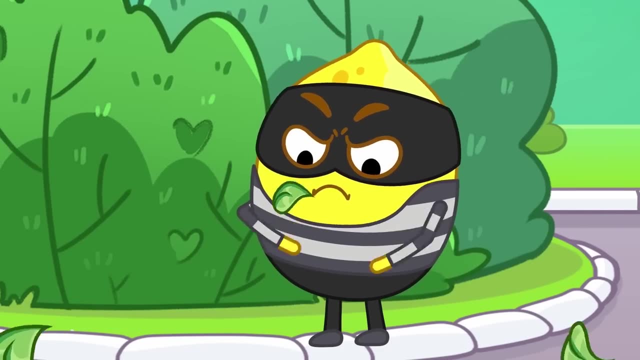 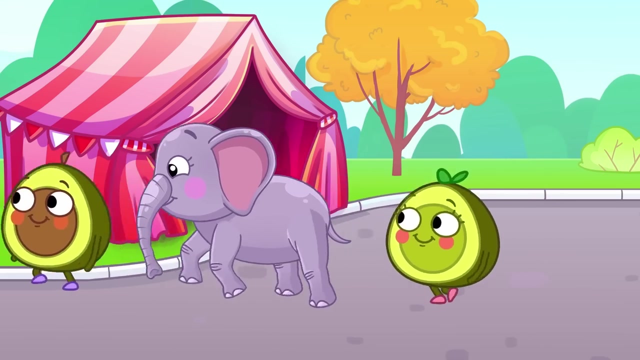 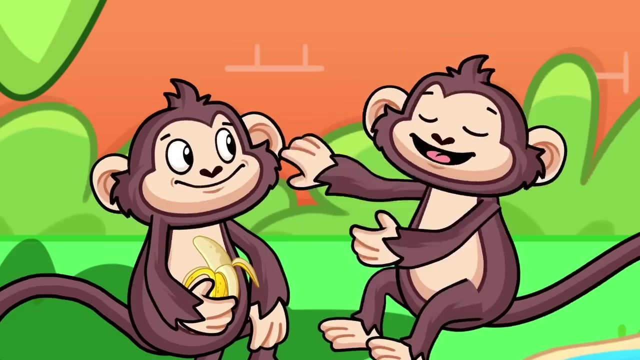 Oh no, Oh no, Oh no, Oh, He must be lost. He's hiding from Mr Lemon. Yeah, We have to help him find his home. Look, Two monkeys by a pond. Maybe your home is here, But he's not a monkey Pit. 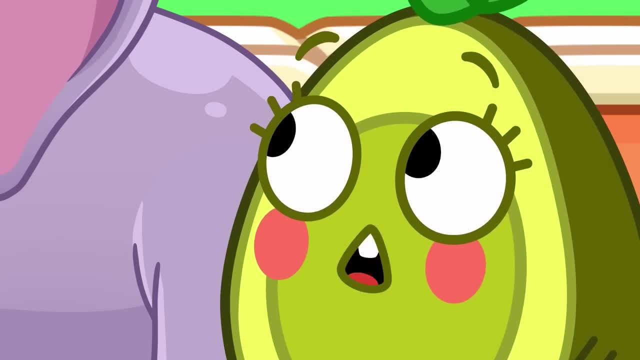 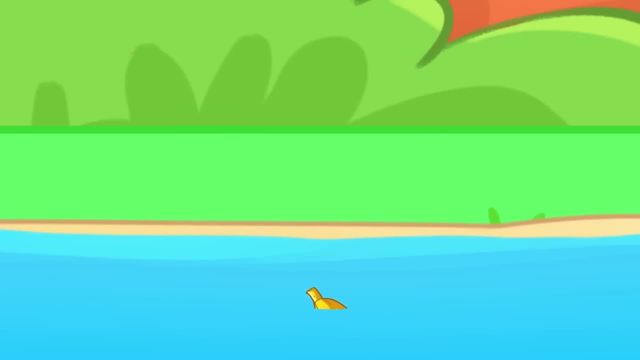 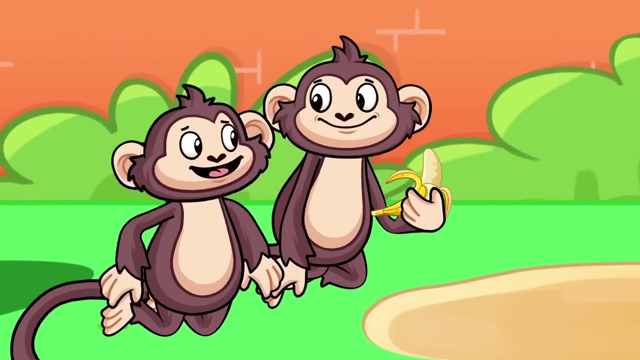 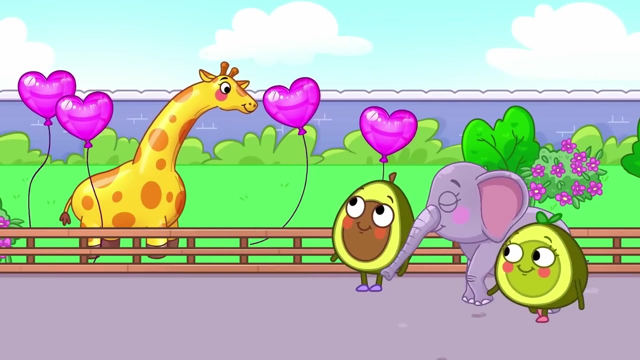 No, They walk on two legs and his walks on four. Oops, The bananas fell in the pond. Thank you, baby elephant. Look, It's a giraffe. Maybe your home is here. I don't think so, Pit. 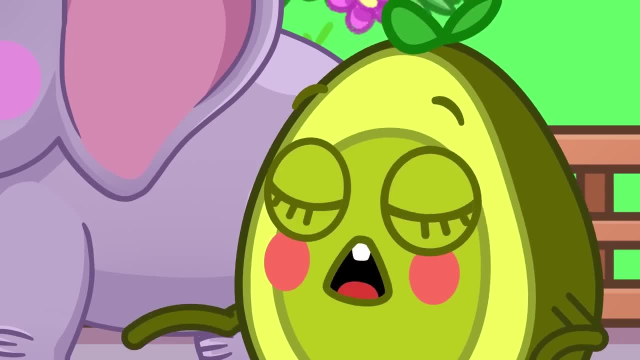 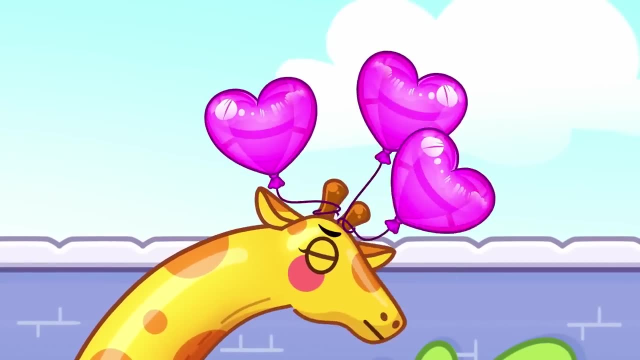 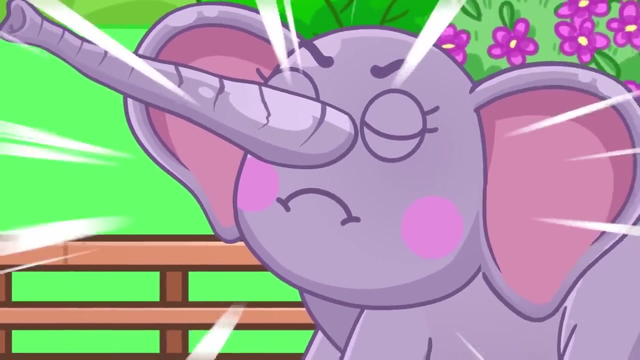 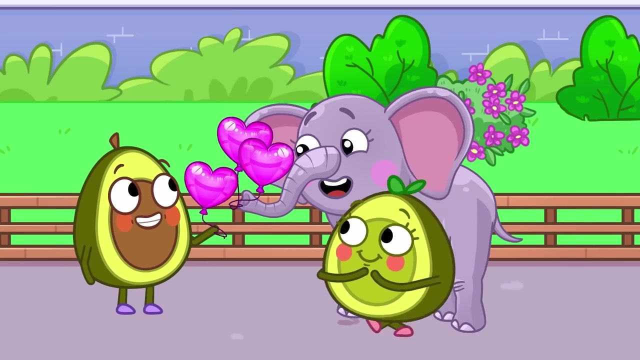 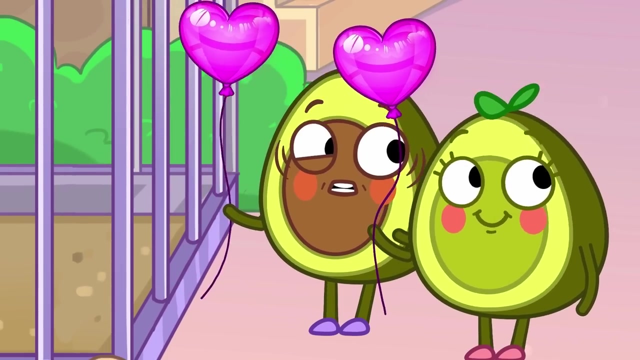 He has a long neck and… Look, They're different colors. The balloons are caught on the giraffe's head. Oh no, He's stuck. Baby elephant helped again. What did you see? Pit, It's Mr Lemon. 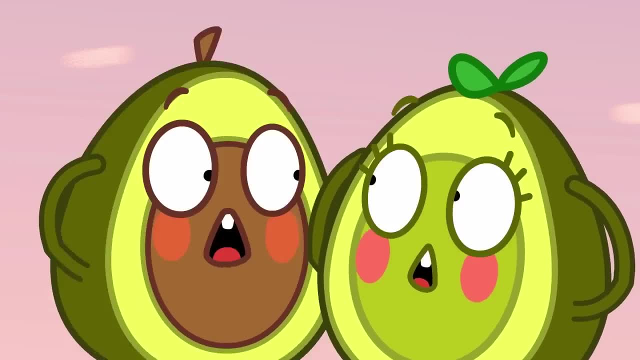 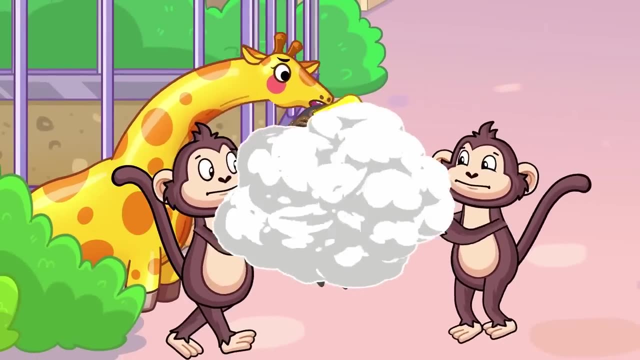 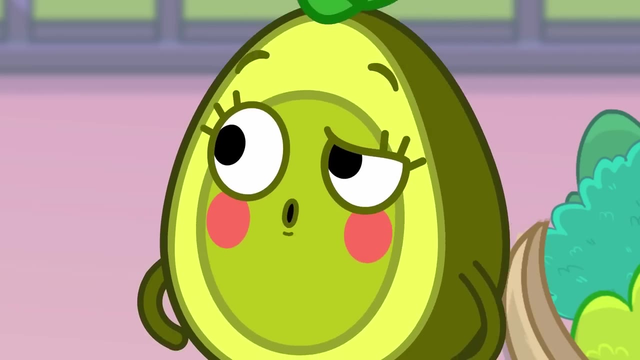 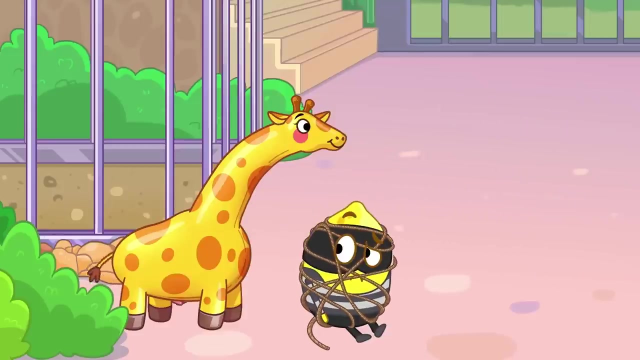 He's back to catch baby elephant. Don't worry, The monkeys and the giraffe will help. Mr Lemon can't hurt baby elephant now. Ooh, Penny has an idea. Now she can search for mommy elephant. There she is. 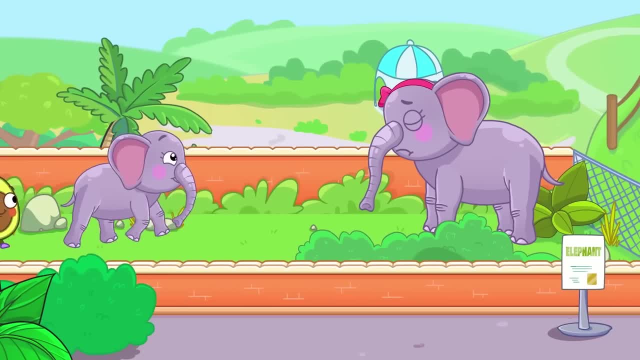 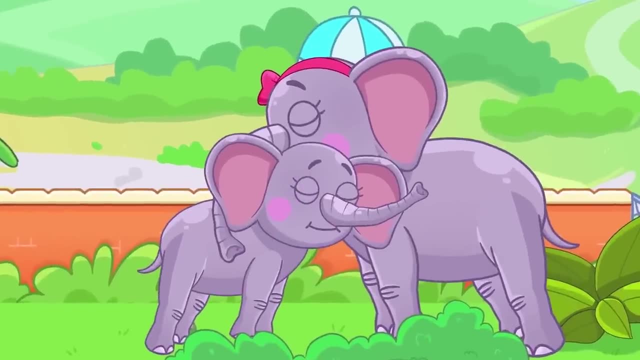 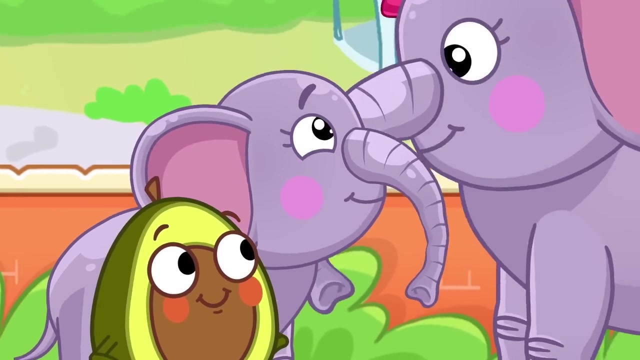 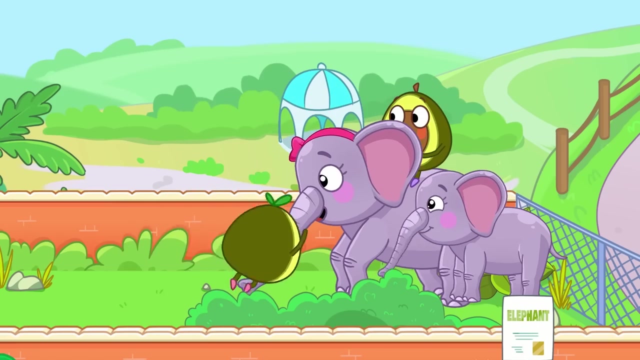 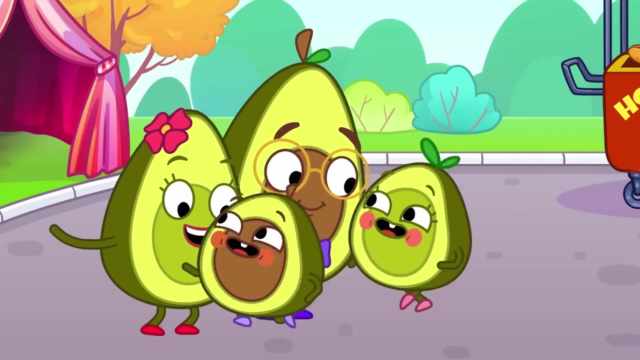 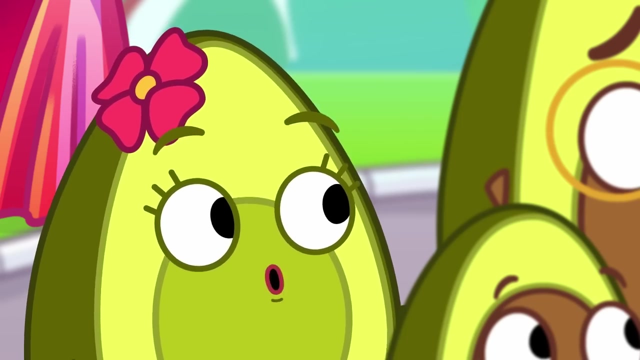 I know where to go. You did it, kids. You found your mom. Now we need to find our parents. There's mommy and daddy. There you are. We were worried. Thank you for bringing our kids back. Now everything is back to normal at the zoo. 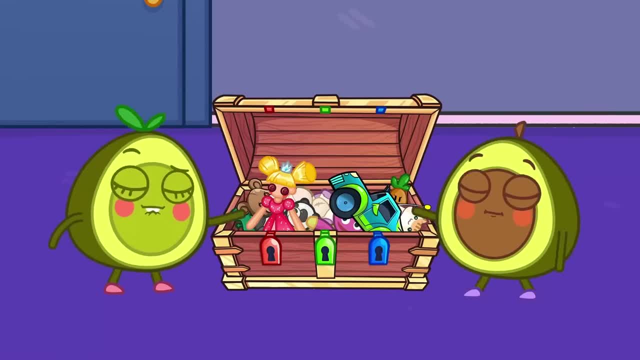 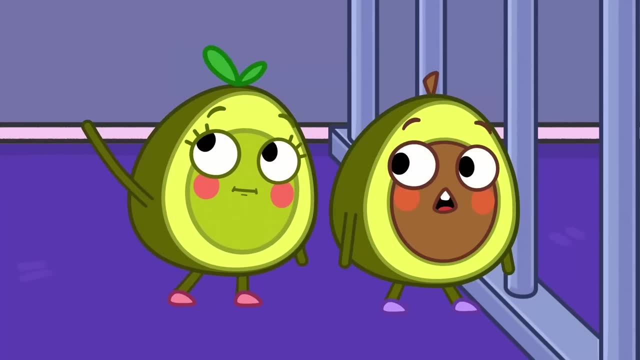 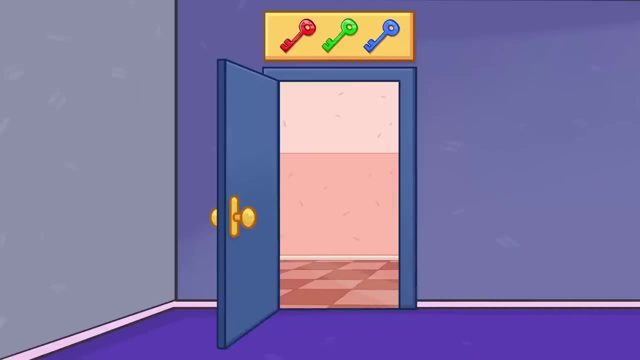 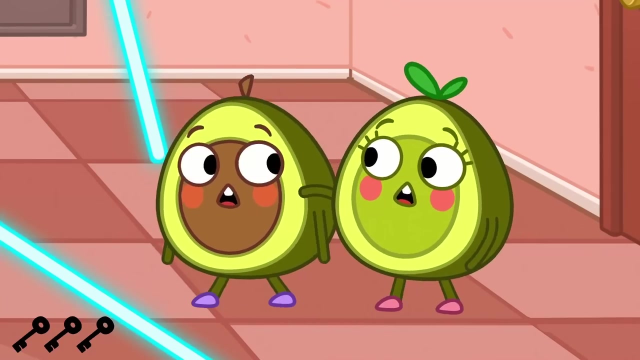 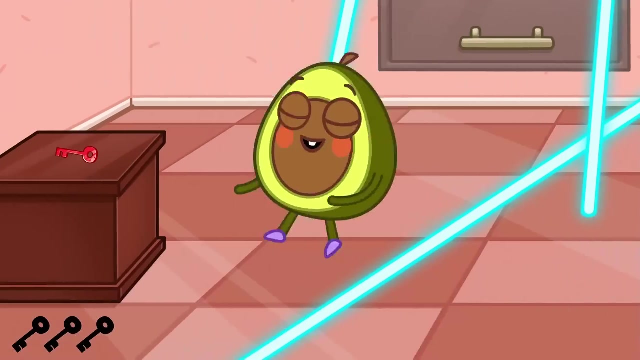 Look, Pit and Penny, A box full of toys. But you're trapped in the room And you need three keys to get out. There's a key: Watch out Lasers, Watch and learn. Yeah Well, Well done Pit. 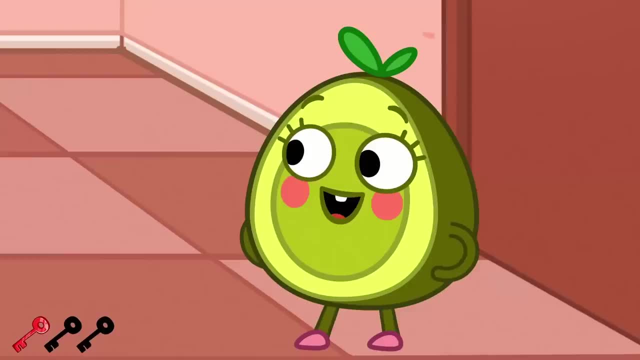 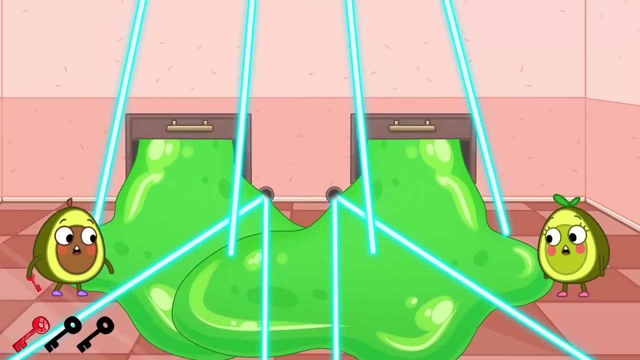 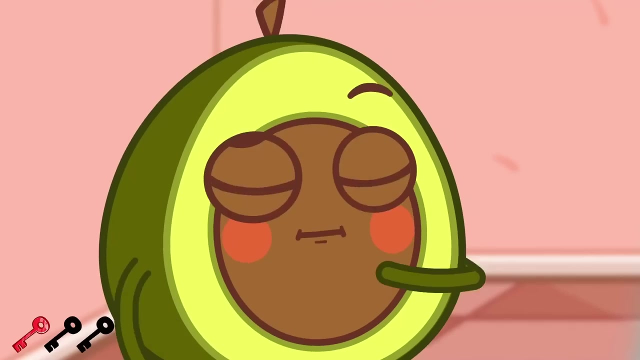 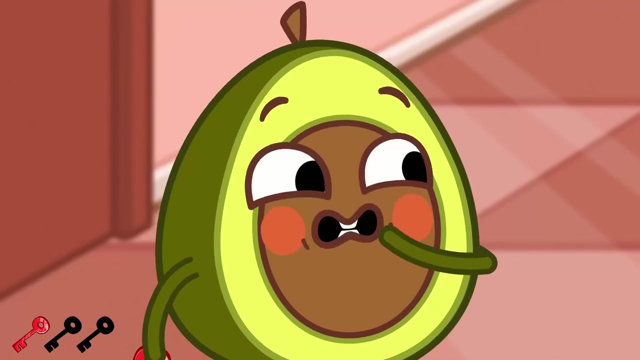 Now you have the red key, But you're stepping on a laser beam. Whoopsie, No, Watch out for the goo, Don't step into this. It's very sticky. Pit has an idea. Grab it Now. Penny can swing a car. 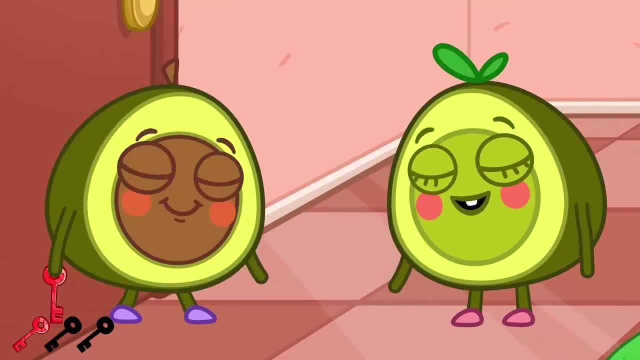 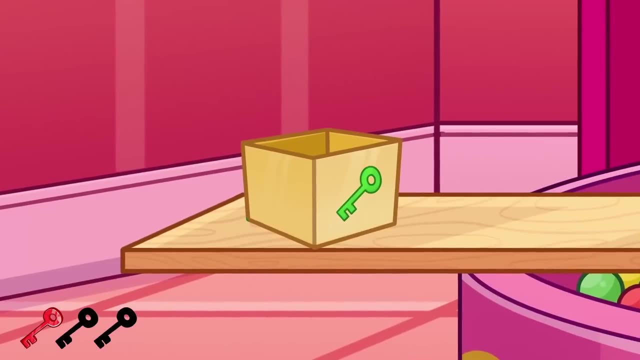 Not a bad idea. The only thing that Penny's got is thecross. Is something stuck in her foot That hurts. Are you serious? Funny? If her verbessaktor comes to help, You can find out everything here Nowサーву. 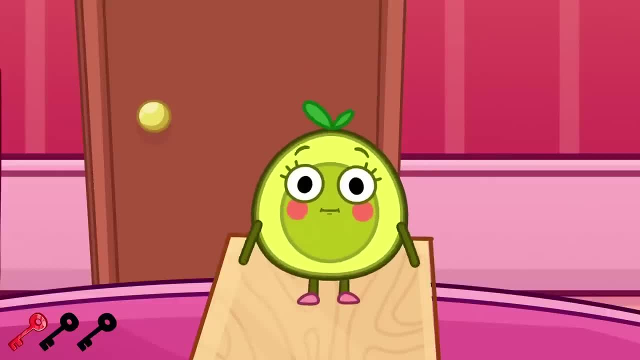 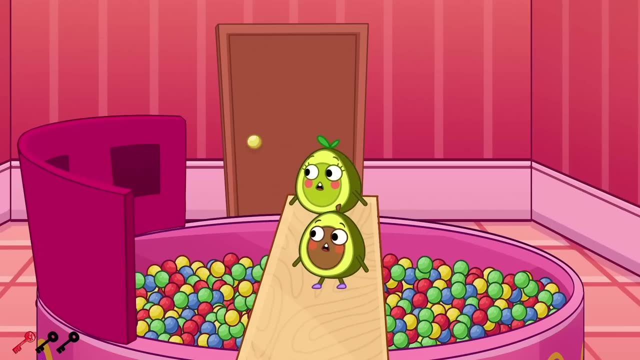 You got an ol' front paw. It's w위 ва АL. You're a dog. Come Goal Time to sleep. А-а Ач, Good night. Good night, Now I've got you Ist. 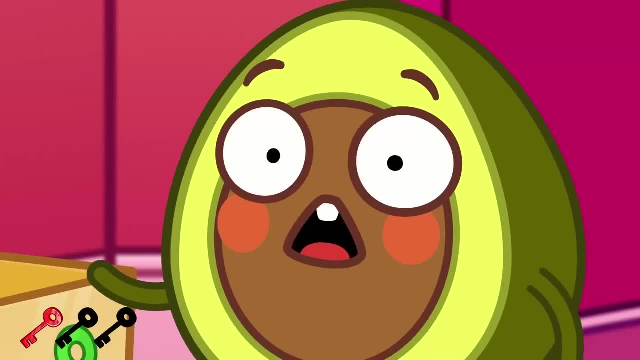 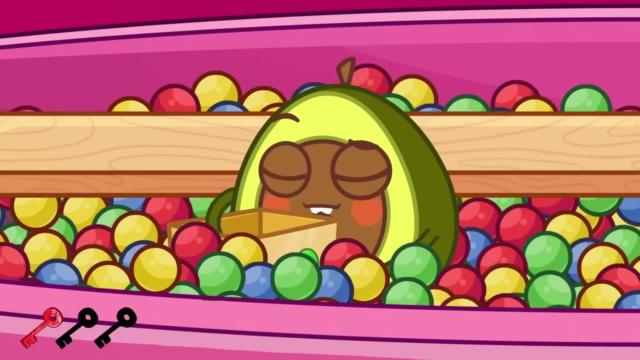 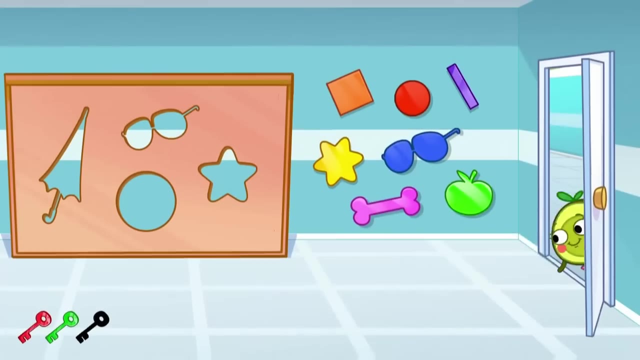 A-a-a Swish, I'm midnight Ngo. A-ah, I don't get it. I'm not made it. oh no, they fell in it lost the keys, but penny found it. it's the final puzzle. we need to find right item. 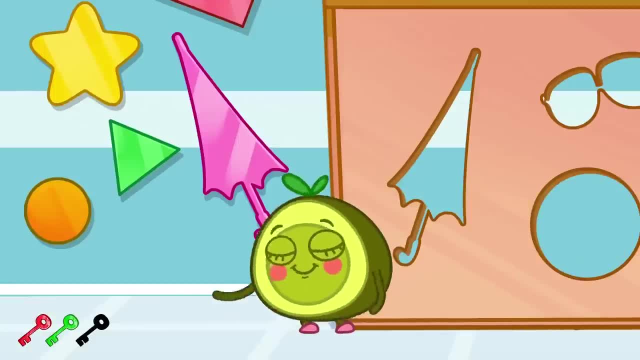 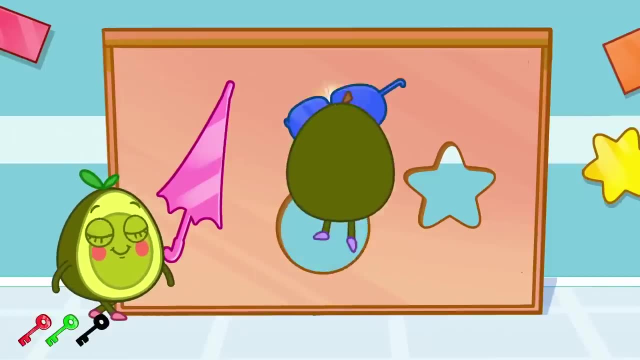 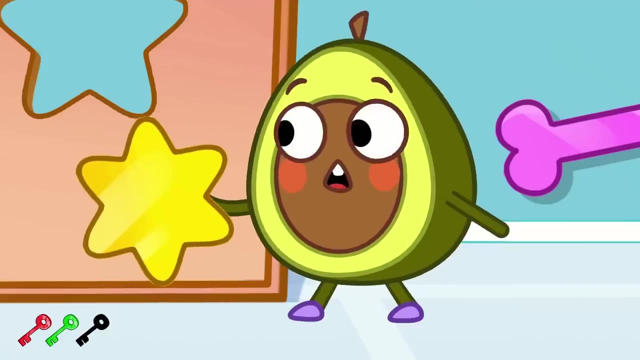 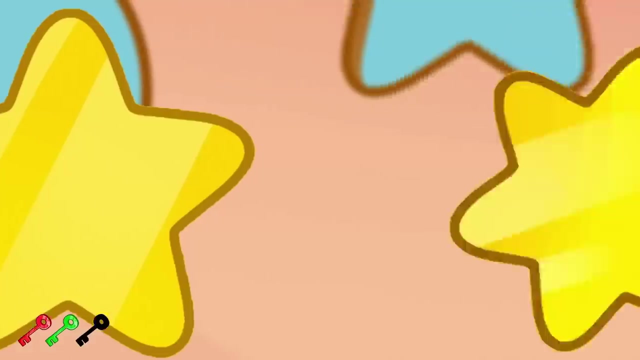 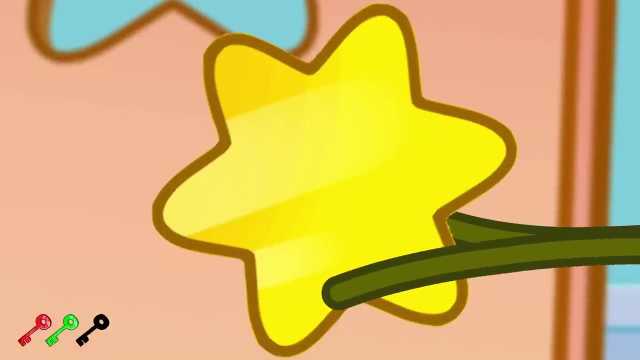 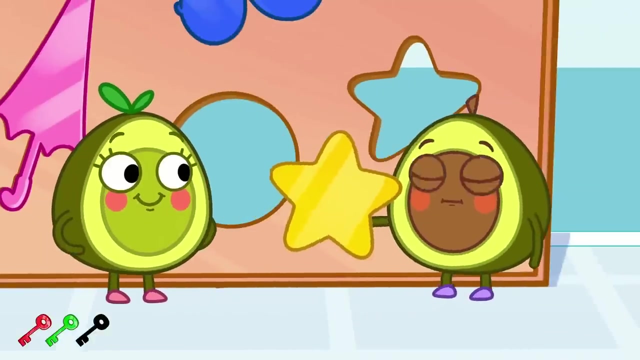 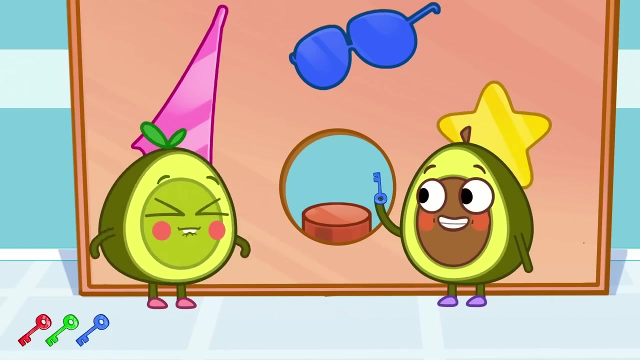 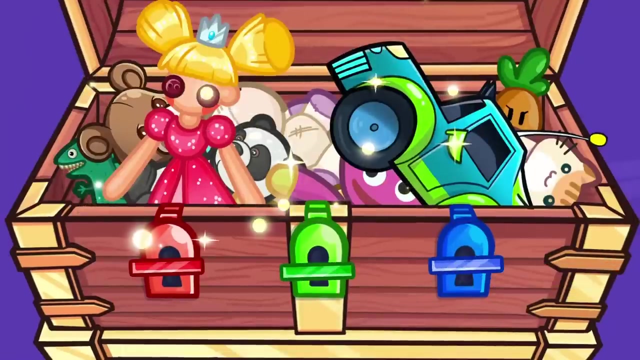 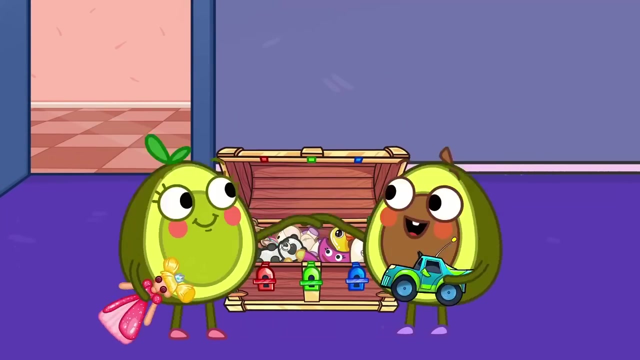 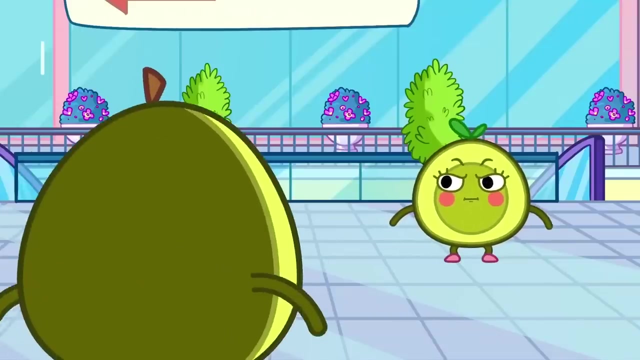 oh, an umbrella, sunglasses. just one more shape. to find which star is the right one, use this one. count the points: pit one, two, three, four, five, six. it's this one. it's the blue key. you can choose a toy. have fun. pitt and penny. penny has challenged pitt to a contest. 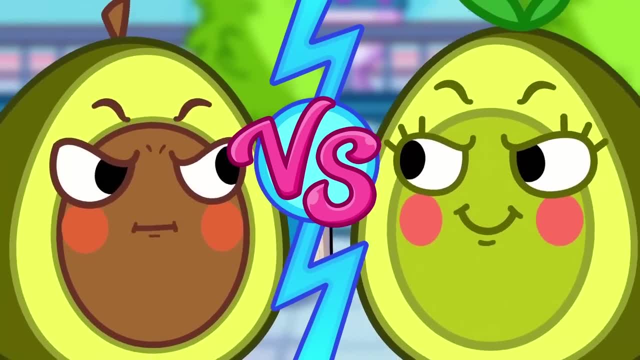 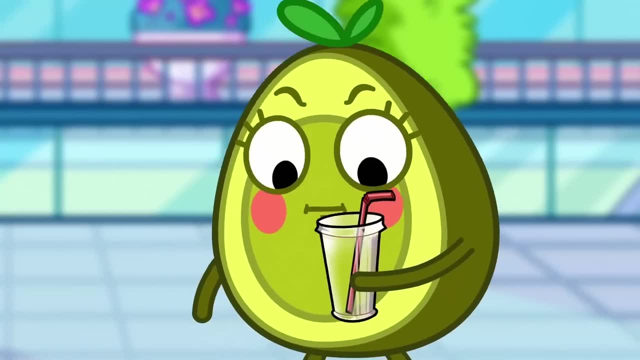 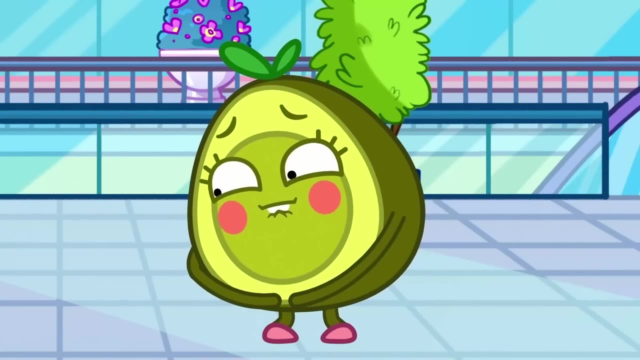 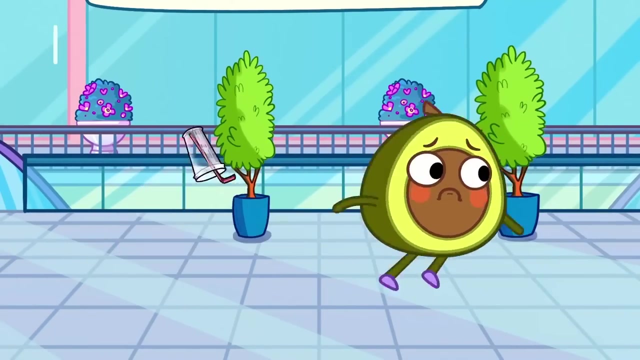 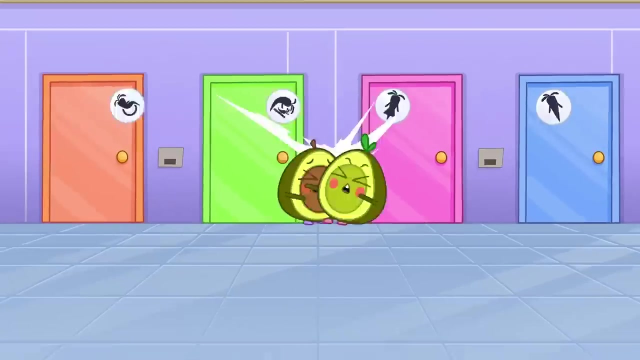 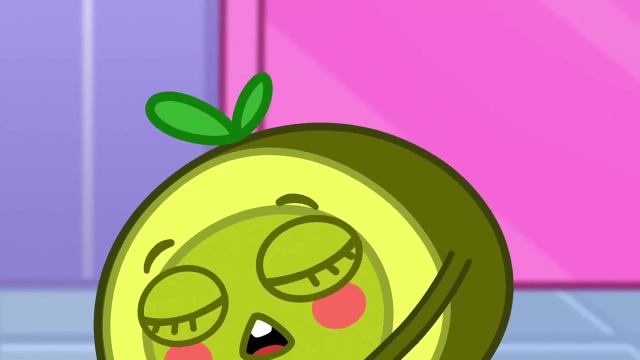 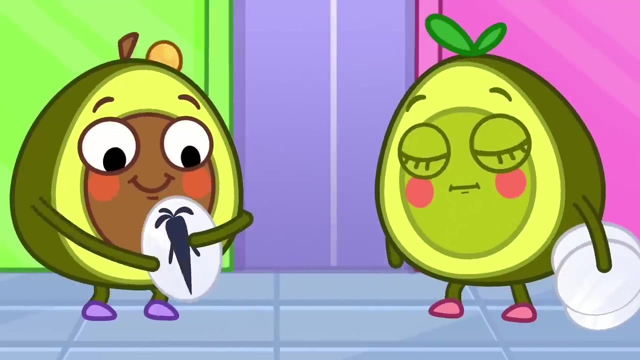 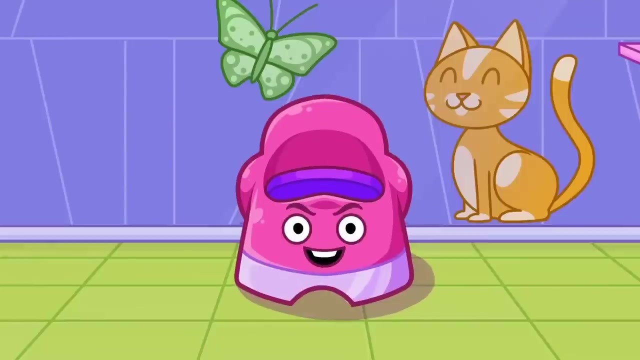 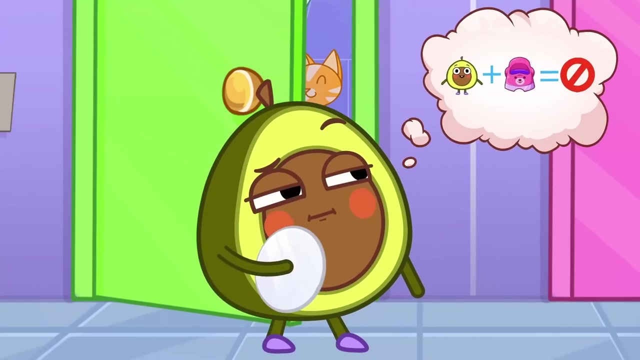 who can finish their drink fastest and go. i win. now penny needs a restroom and pitt does too careful kids. the restroom signs are all mixed up. where does this sign go? where does this sign go? where does this sign go? fake, according to it? just here, can i. 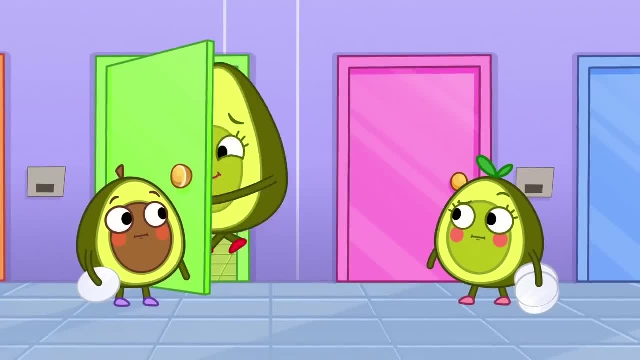 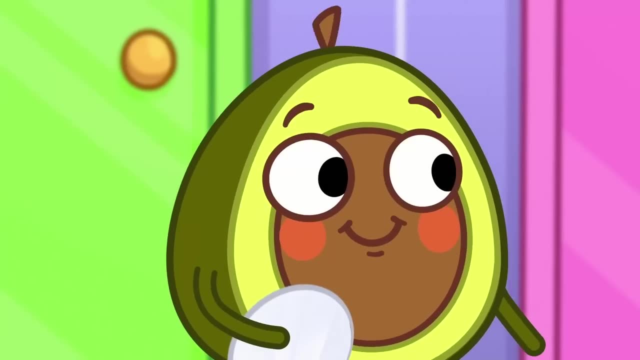 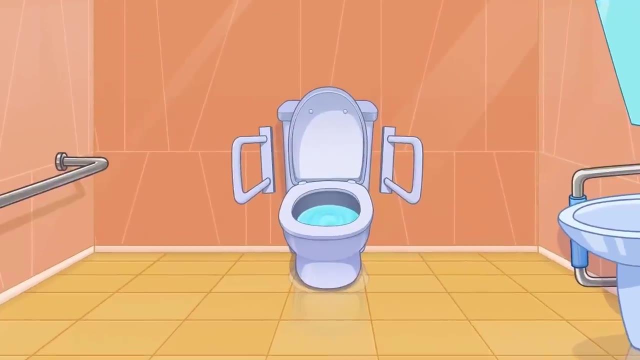 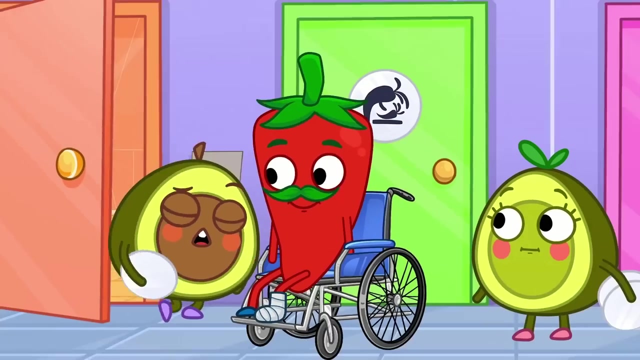 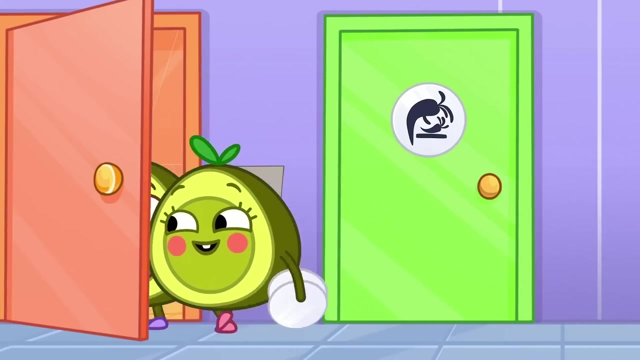 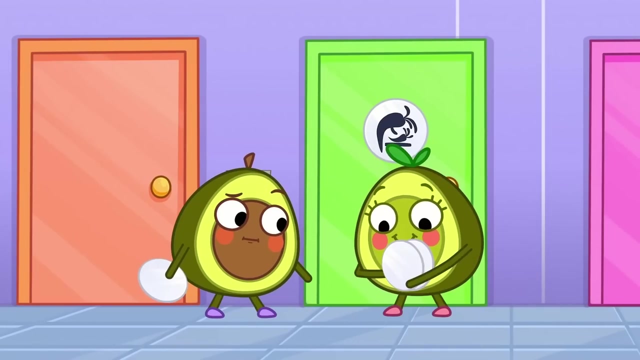 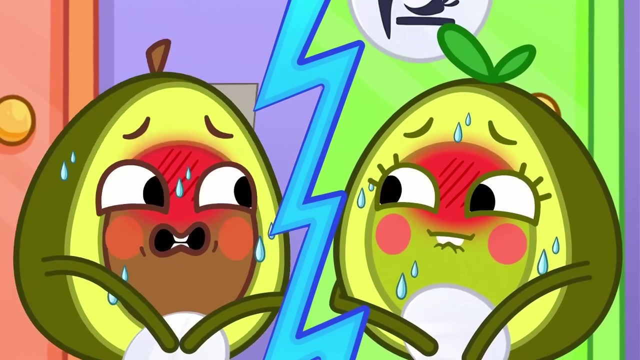 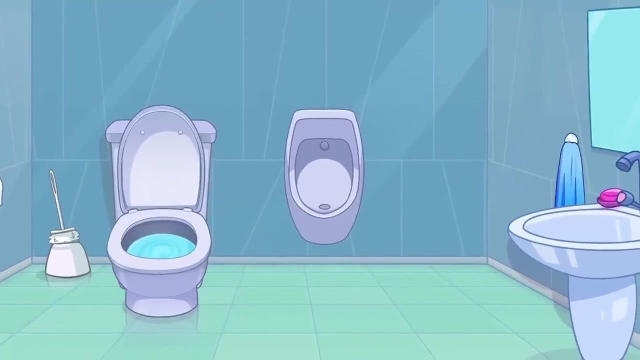 see you come search me hide. so here, no note, Come here, my friend, Weep it. It's the handicap toilet. And what sign goes on this door? The handicap sign. Good job, You two. better hurry Attention, The girl is here. 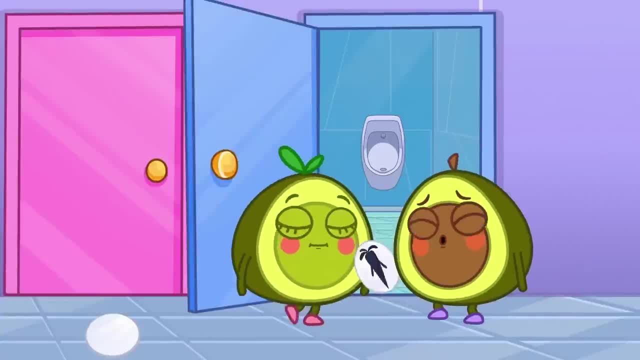 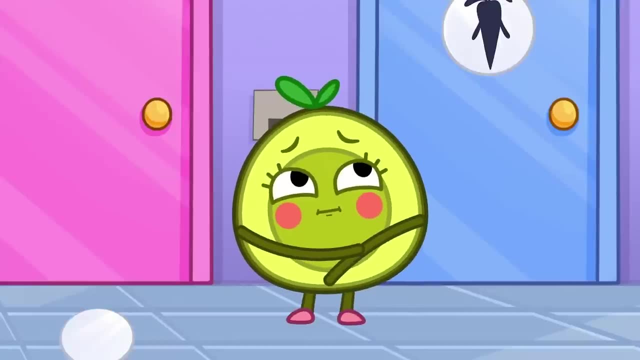 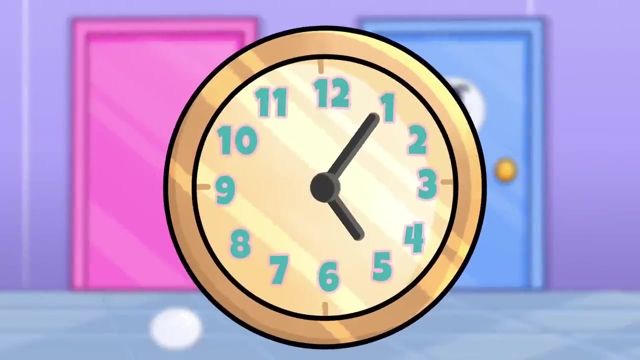 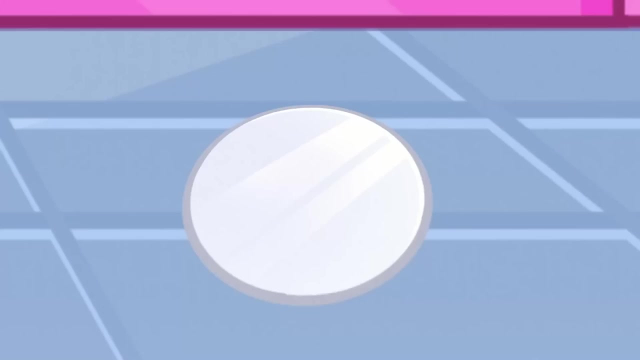 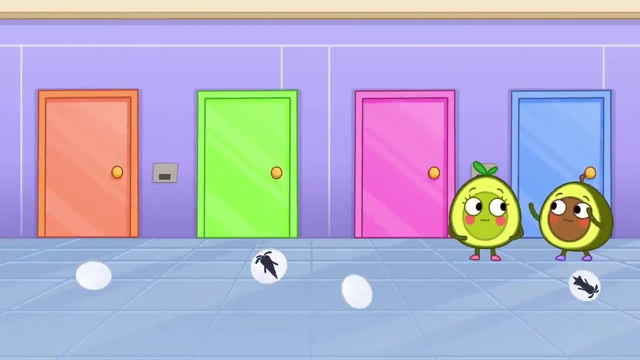 This is where Pit should go. You found the boy's toilet, Thanks. There's one door left, Penny. You forgot one thing, Penny: The sign for the girl's restroom. Oh no, Not again. Pit's dyeing his shoes. 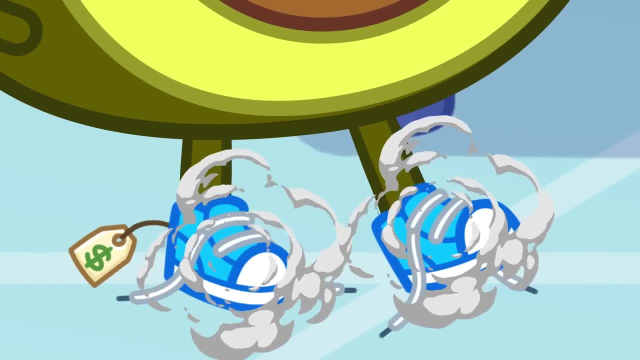 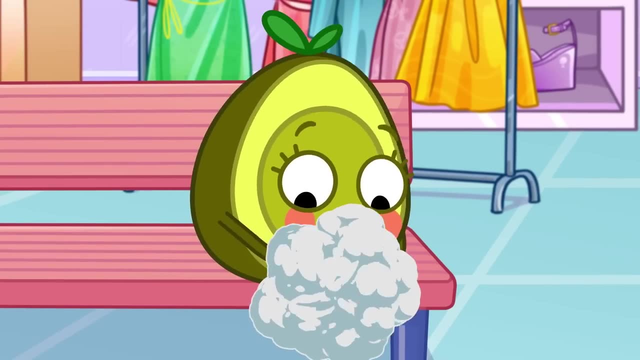 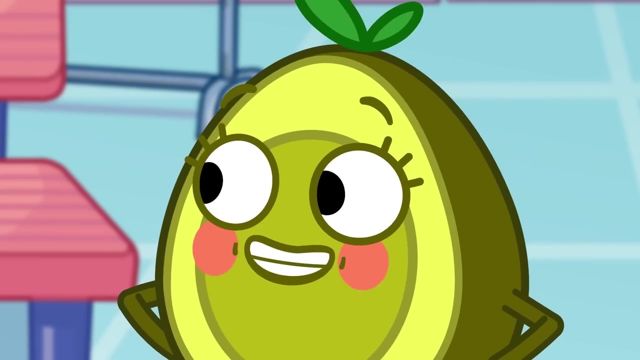 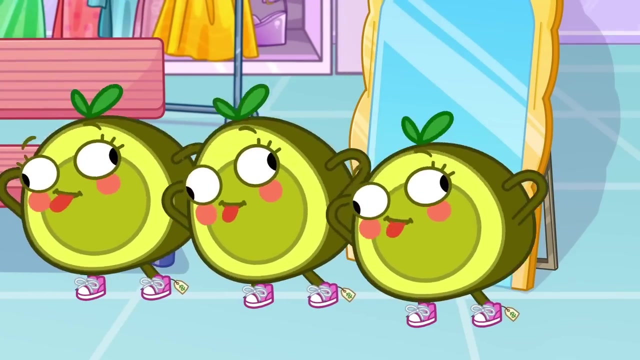 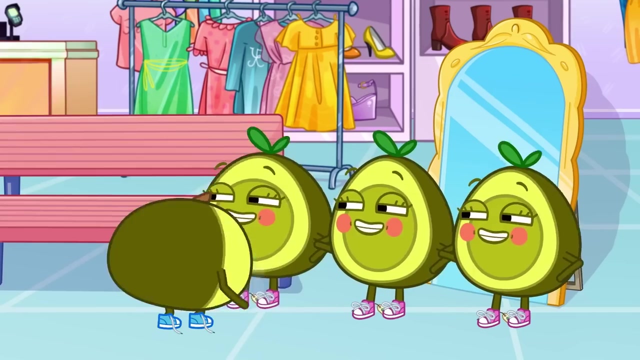 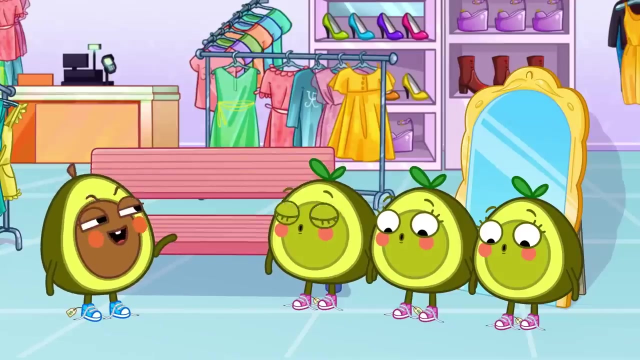 I did it. Oh no, They have come undone. Can you do it, Penny? Hmm, There are three pennies. Pit will find the real one. Let's test your skills. Which penny? Penny can tie her own laces. 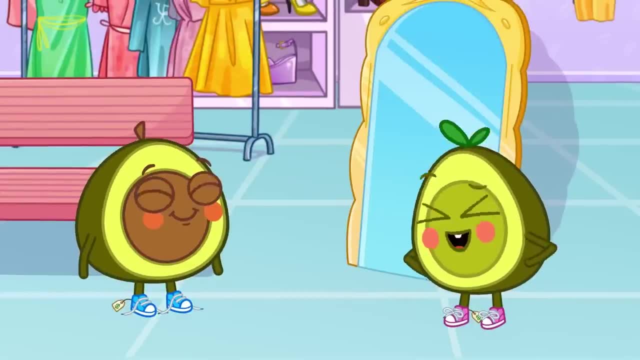 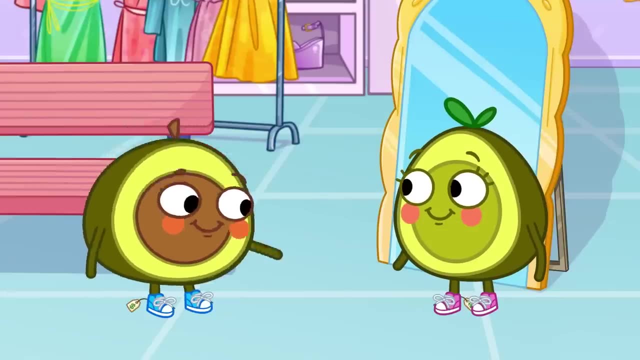 This is the real penny. I'm not that bad, am I? I'll buy it If you want. Let's see what we can do. Oh no, You're not that bad. I'm not that bad. I'm not that bad. 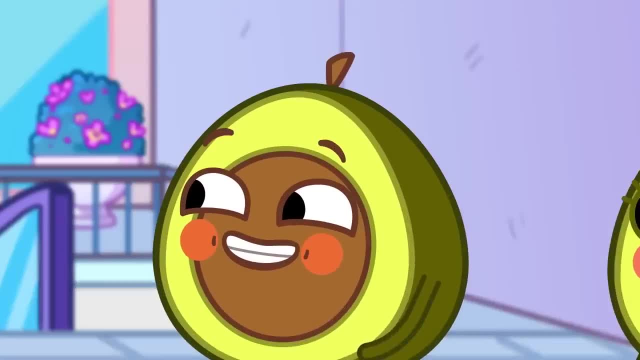 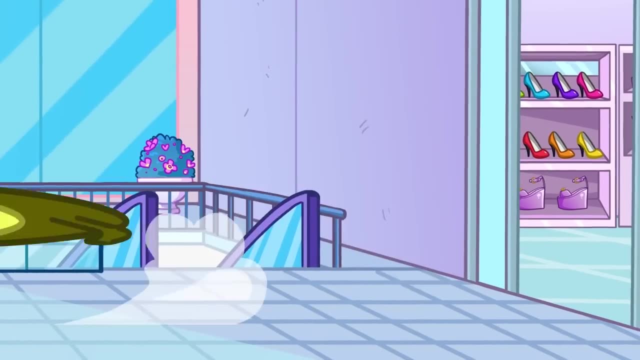 What a good boy. Okay, let's go. I'm not that bad as a child. Whatever, Let's try in the car. No, No, Stop, No, No, Stop, Stop, No, No. You're the only one in my car. 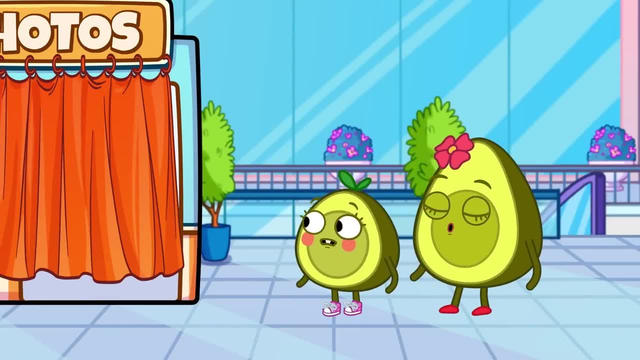 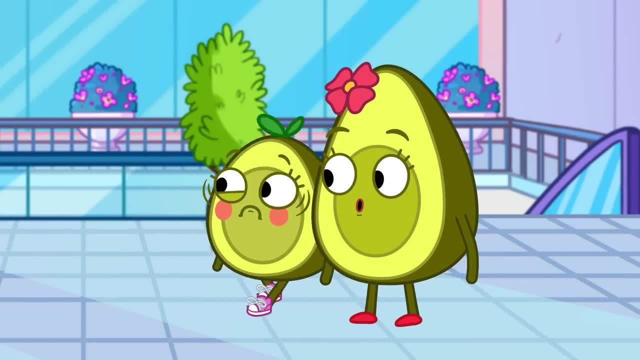 You're the only one in my car And I can't get away. No, you're not the only one. You're the only one in my car. No, No, Oh, No, No, Which is the real pit? You can do it, Penny. 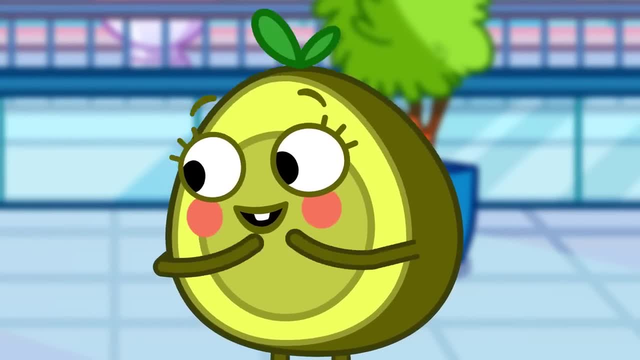 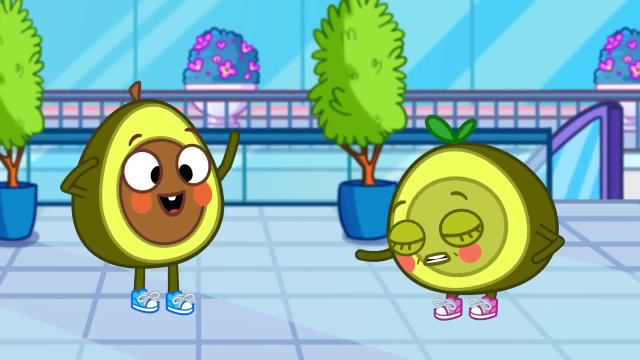 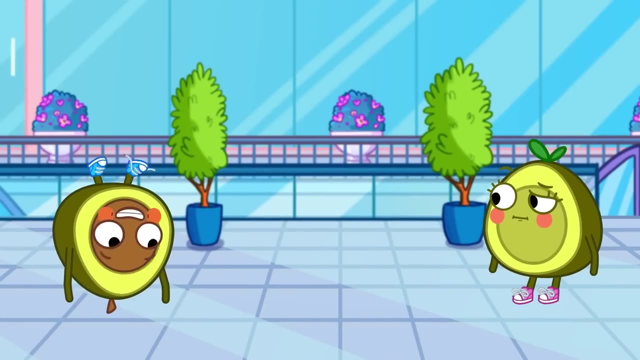 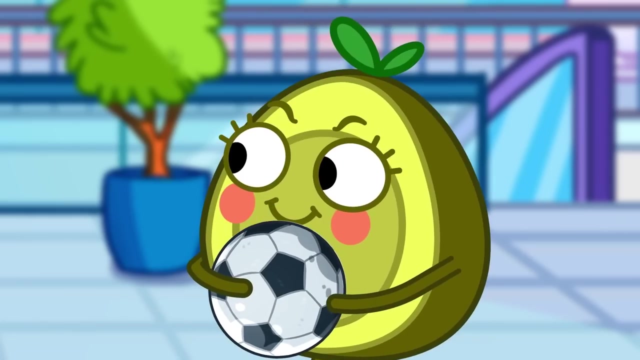 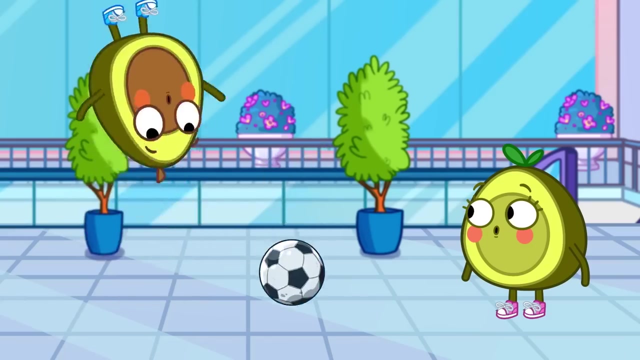 Hey, Can you do that? What do you think, Penny? No, no, no, My brother is not a prankster. Let's check your skills. Let's see what you've got. Can this pit play soccer? No, no, no, My brother is not clumsy. 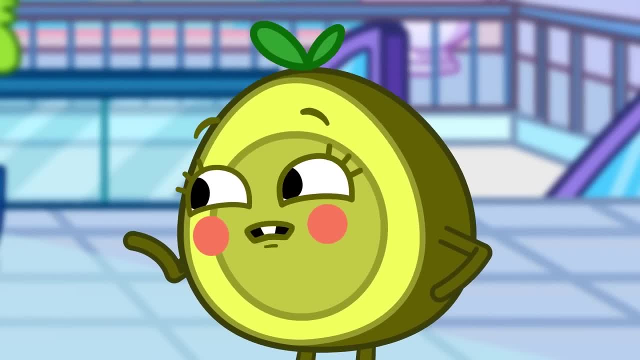 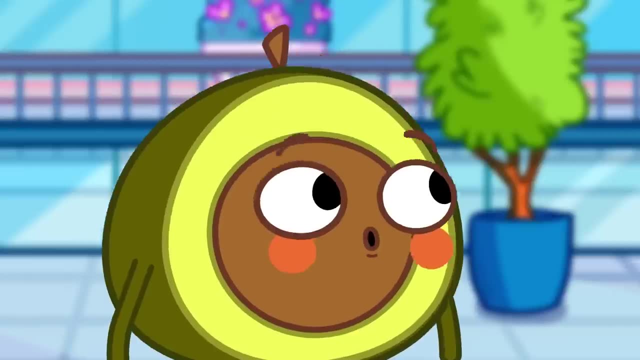 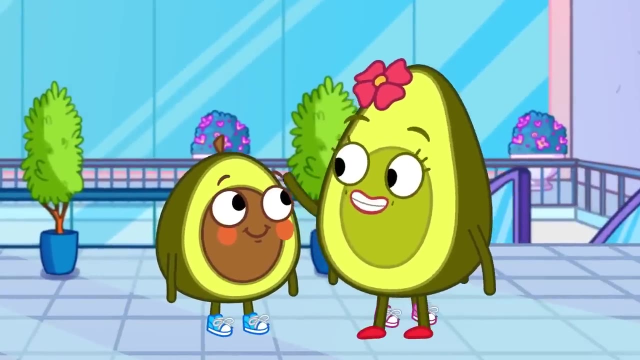 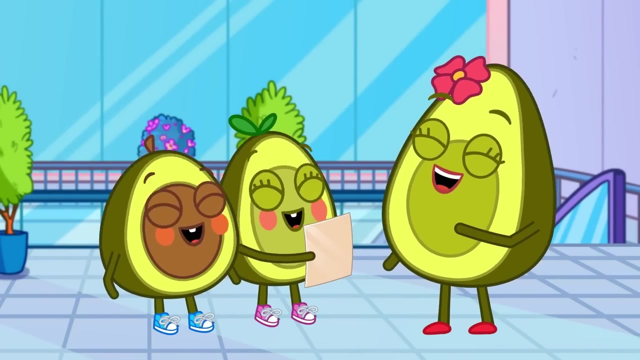 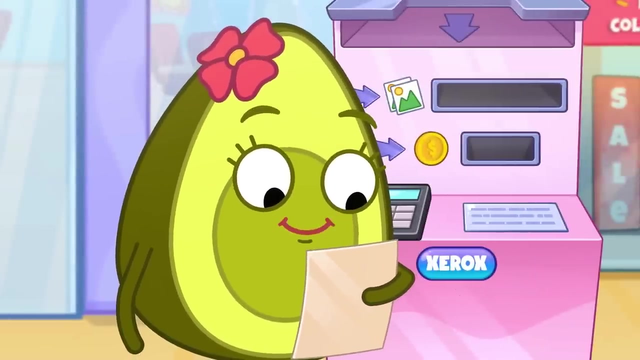 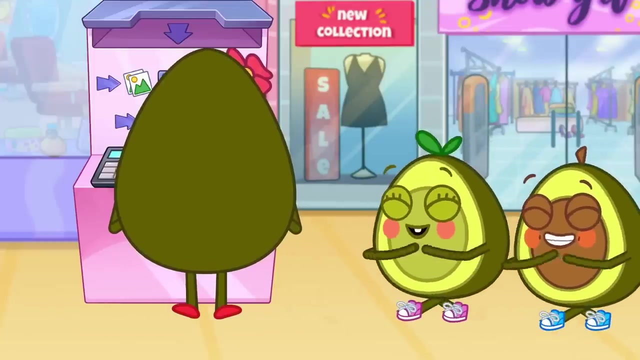 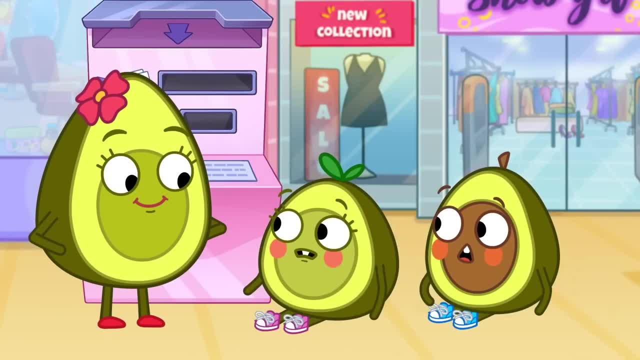 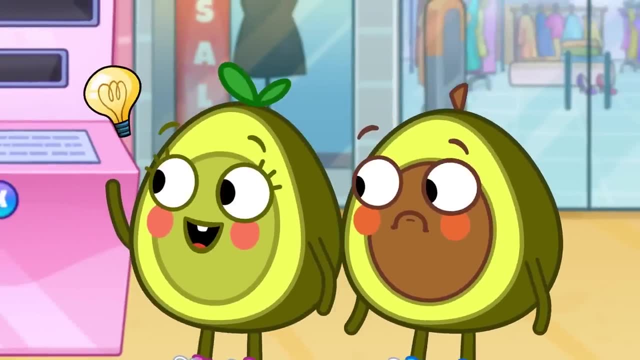 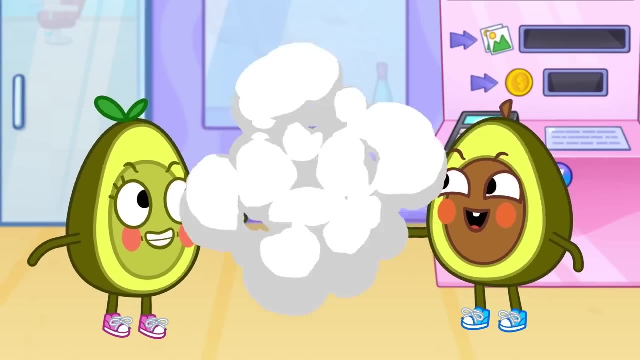 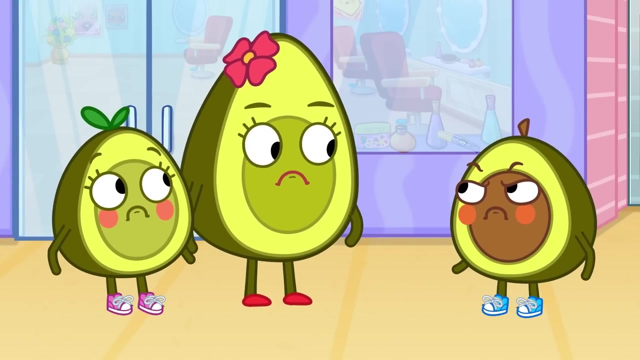 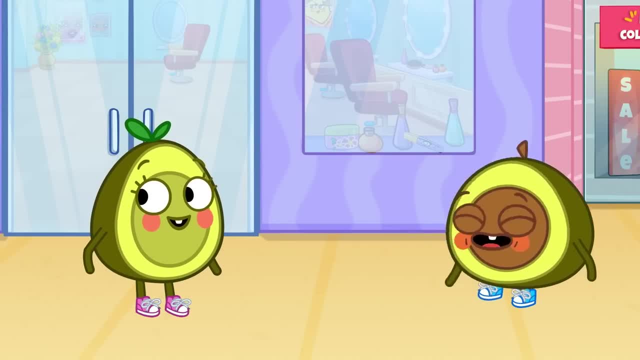 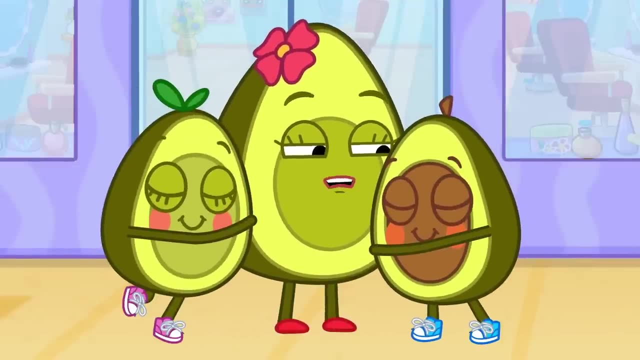 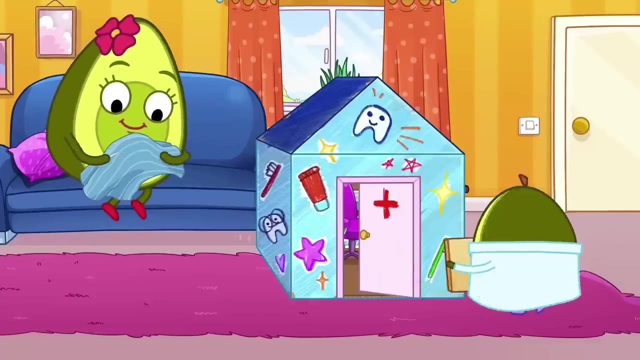 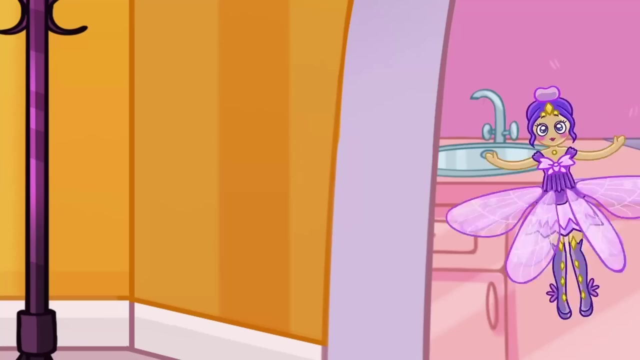 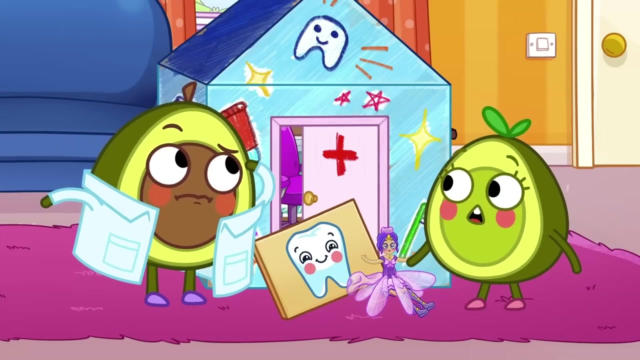 Mom, Mom, They found her. I'll not confuse you with anyone else. Pit is pretending to be a dentist And he's ready for his first patient. Stop, No Wait. Penny's doll has a bent wing. It needs to be fixed. 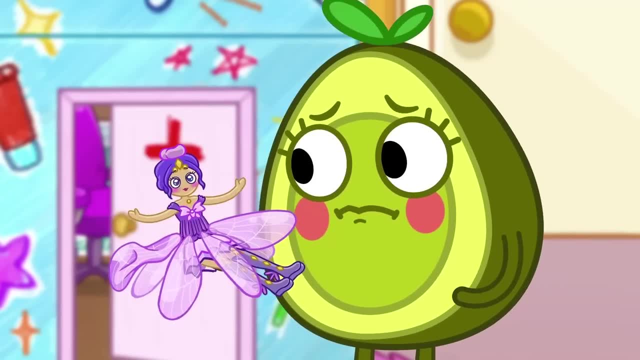 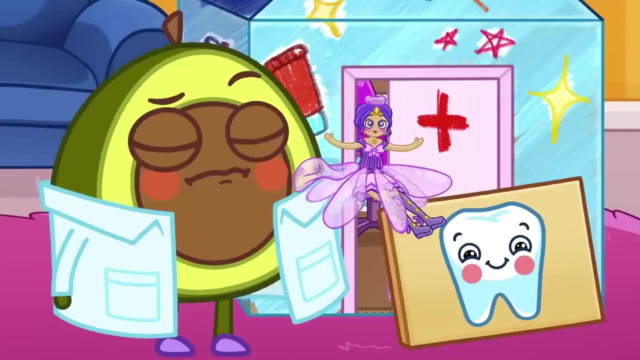 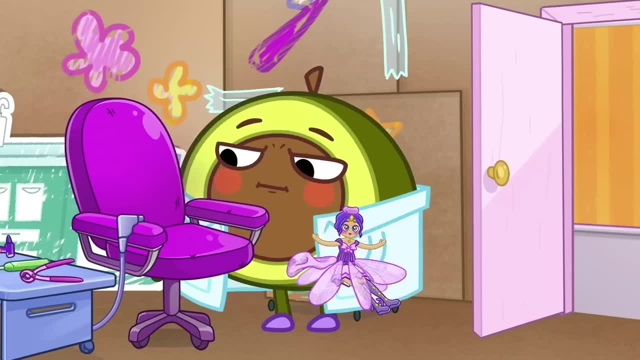 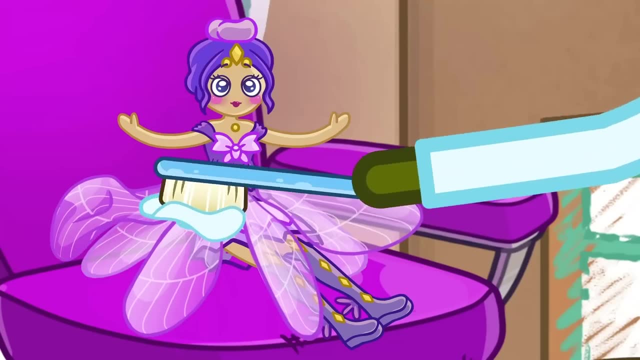 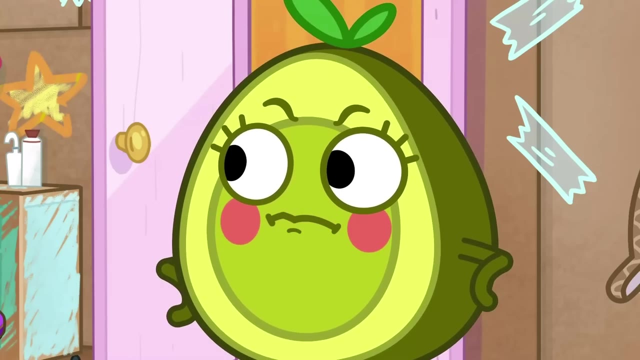 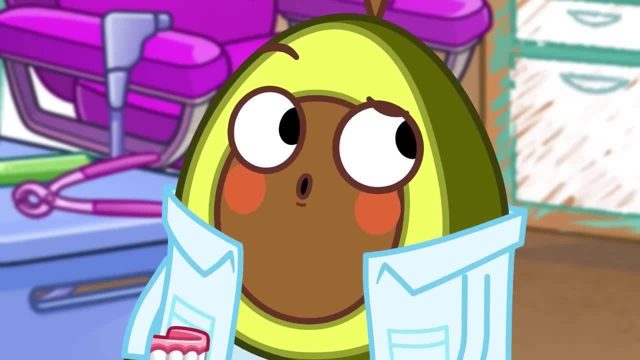 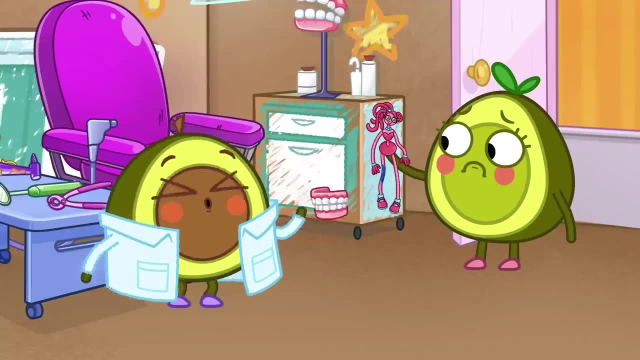 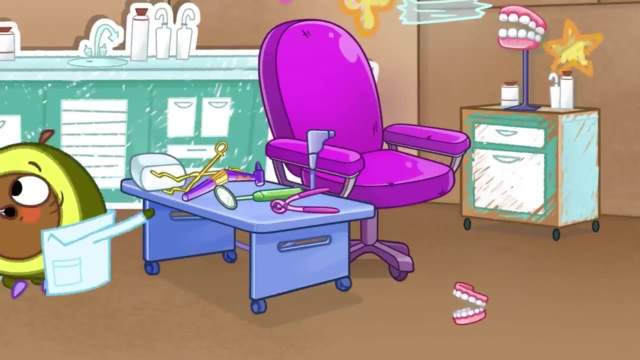 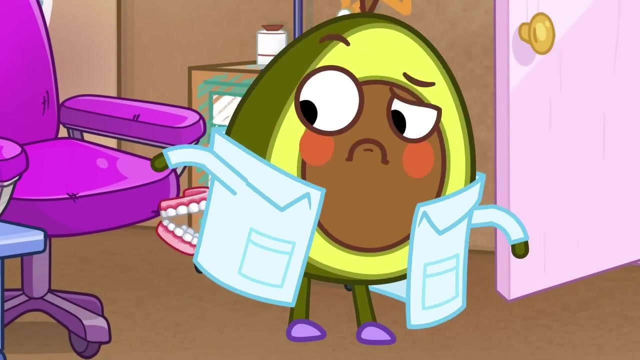 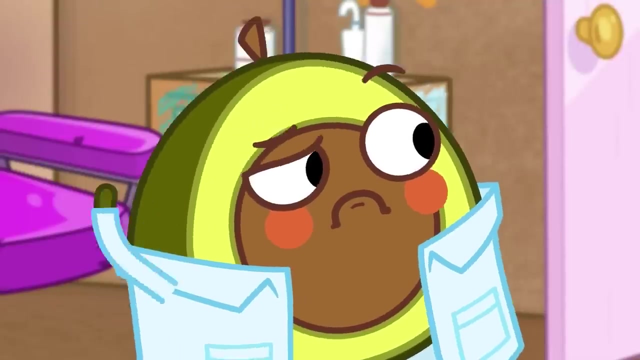 Oh, Pit, You're making it worse. Pit's waiting for another patient, Pit. She has a boo-boo. That doll has a stain. Watch out, Pit, Poor Pit. Will you help Pit? He has an idea. 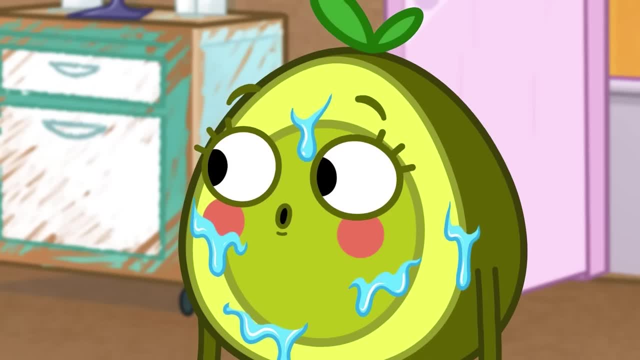 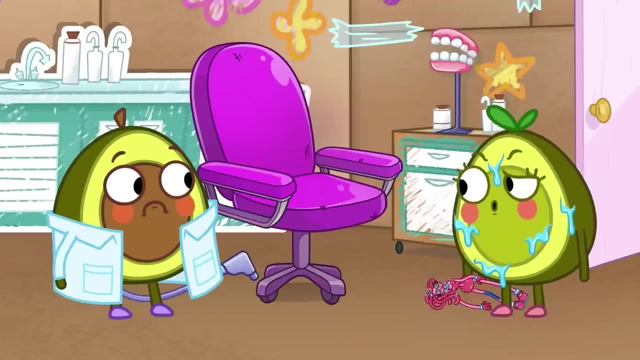 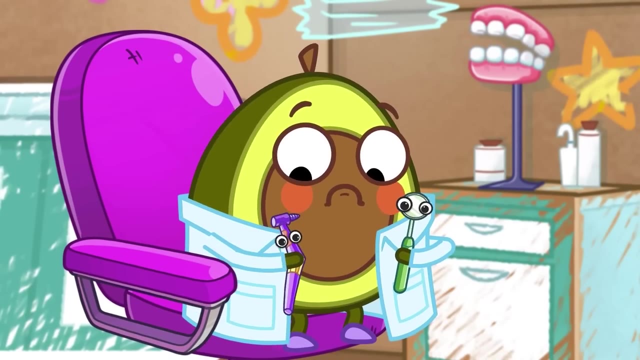 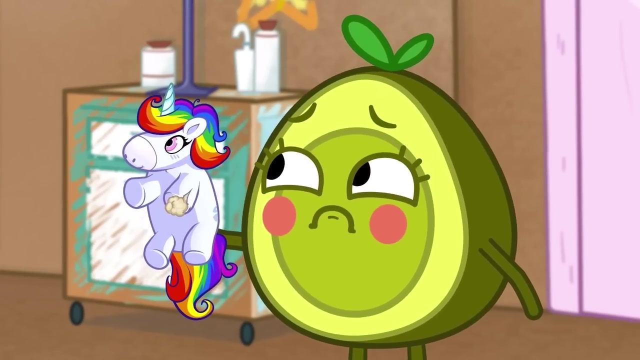 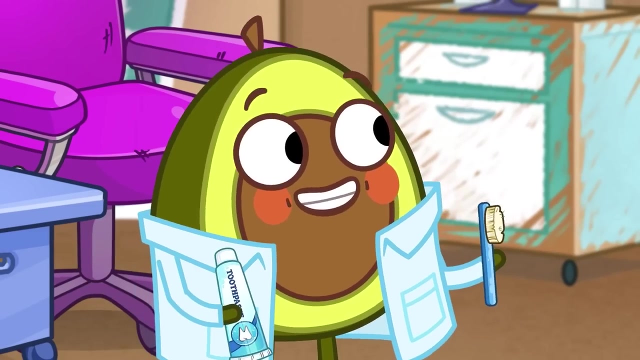 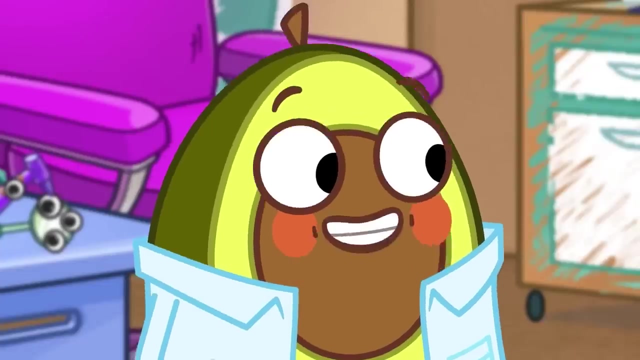 He thinks water will help Pit. the doctors don't do that. Pit really wants to help someone Save her. I don't know any other doctors. Can a dentist fix Unicorn's leg? Not again. Penny's afraid of a dentist's tools. 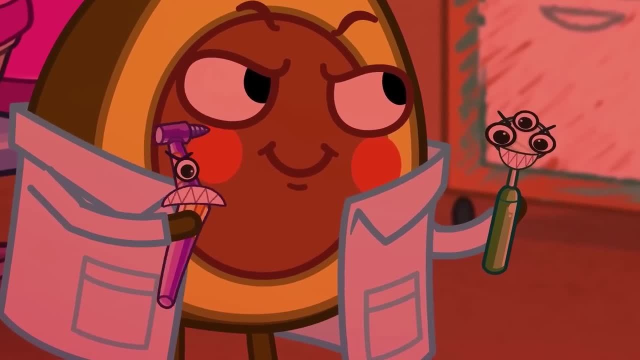 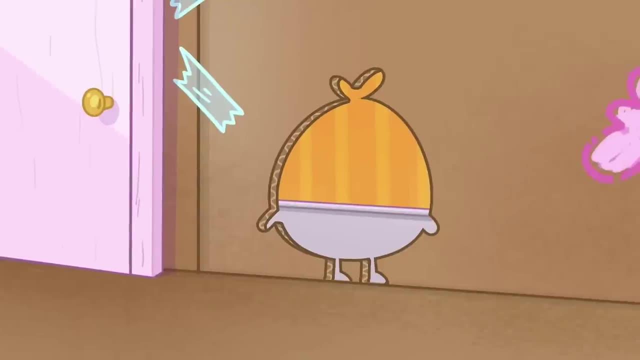 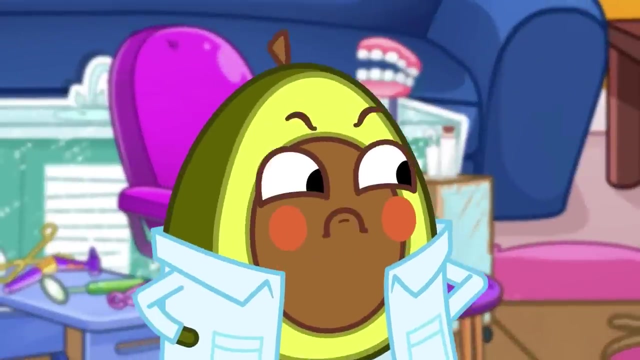 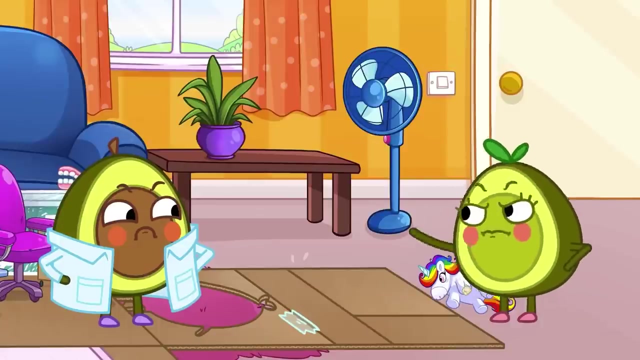 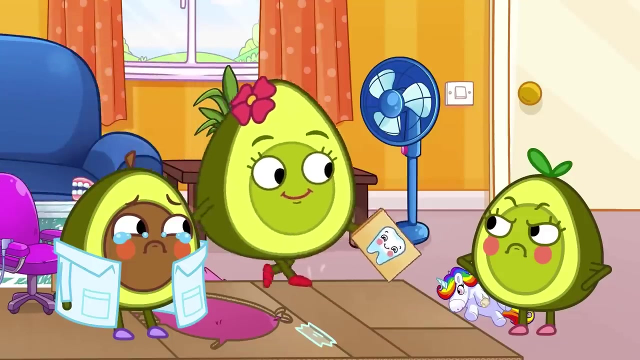 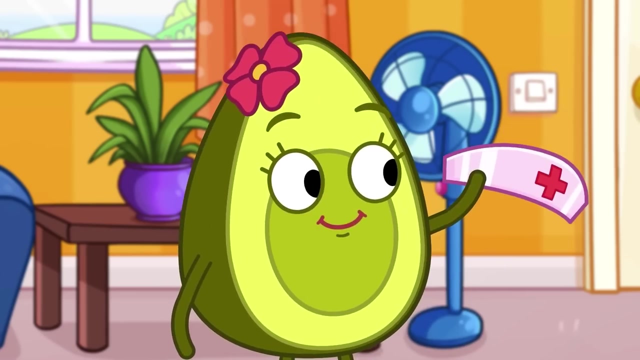 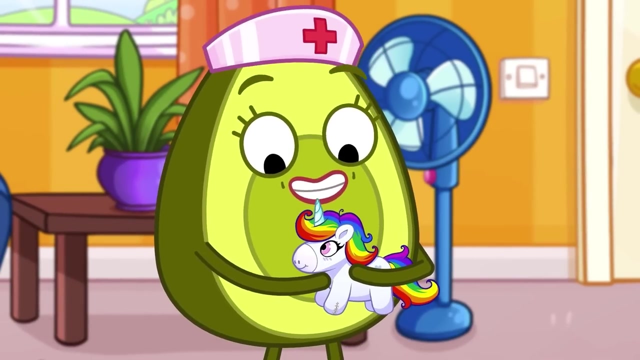 She thinks they're scary. Oh, Pit's office fell apart, It's because you're a bad doctor. That wasn't very nice. Penny Pit is a dentist, He only treats teeth. Now Mommy is a doctor. All doctors are different. 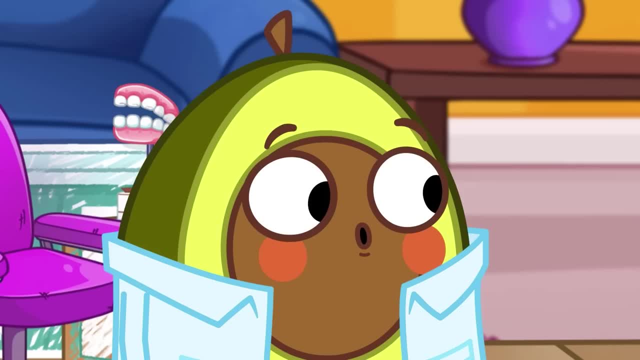 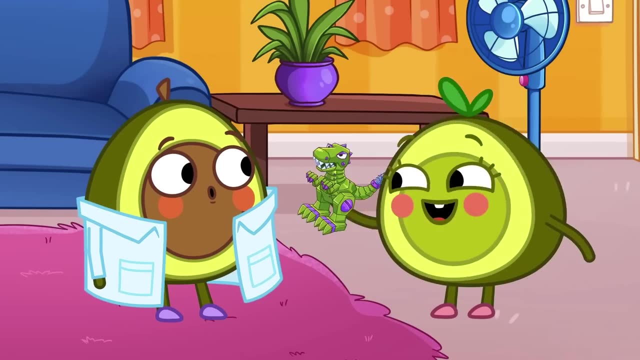 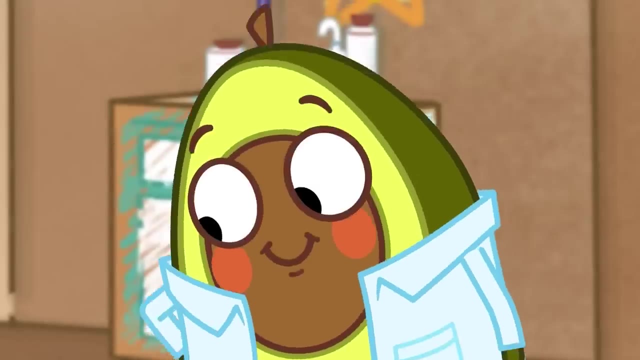 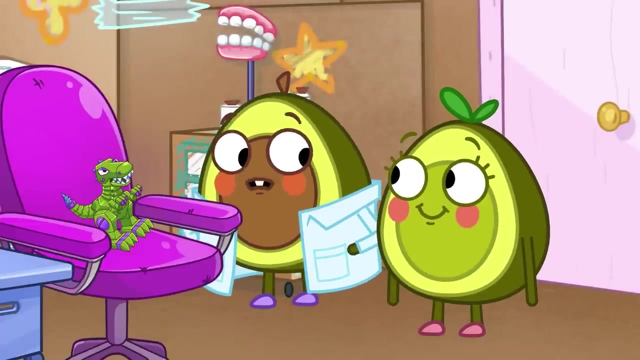 I'm sorry. Pit Penny knows the perfect patient for a dentist. T-Rex has lots of teeth. First Pit examines the teeth. He hasn't brushed his teeth in a while. If you don't brush your teeth every day, you'll get a toothache. 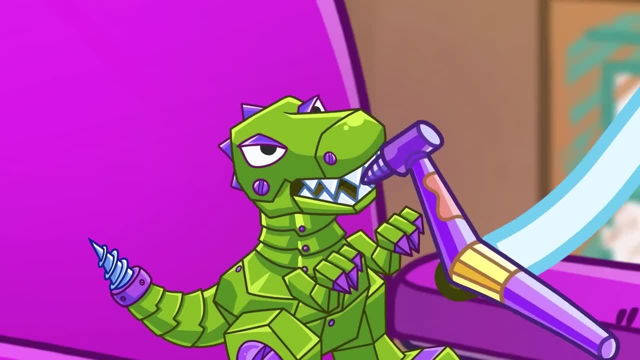 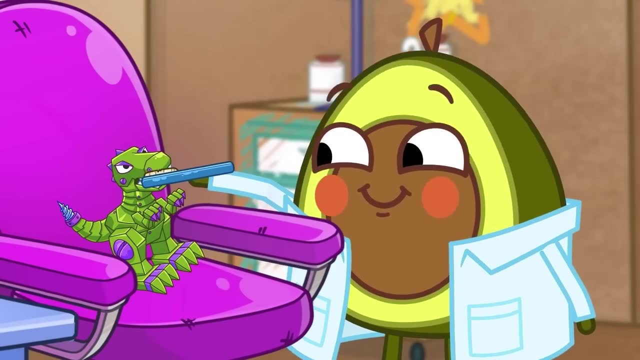 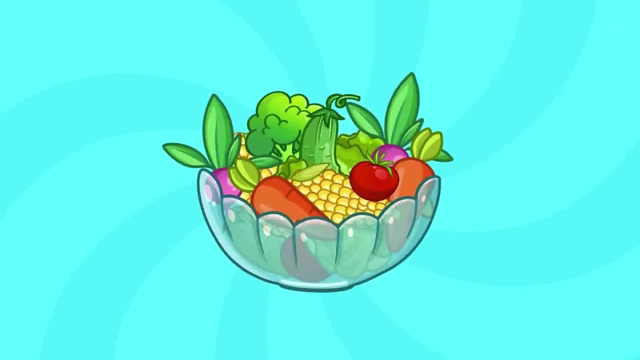 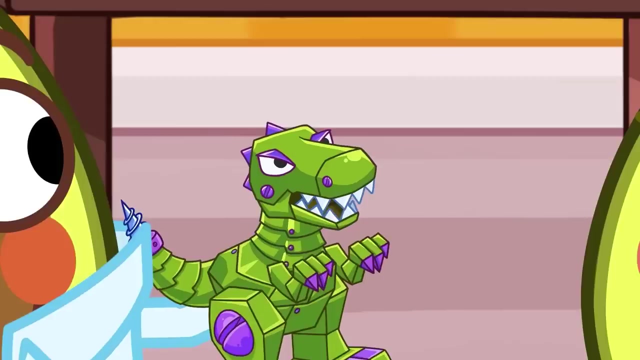 You'll get a toothache Every day. They may get sick. A dentist will then help clean them. Remember, Brush your teeth and eat more vegetables than sweets. Vegetables are good for your health, But sweets can cause cavities And your teeth will be healthy. 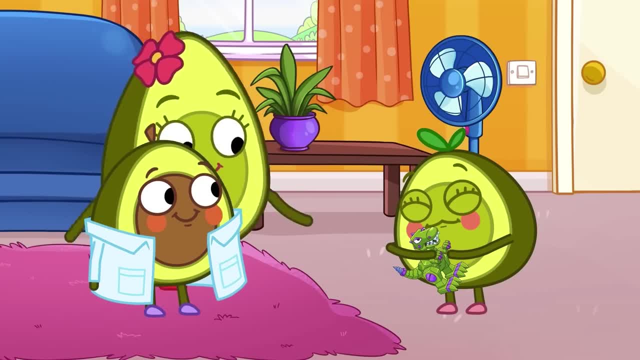 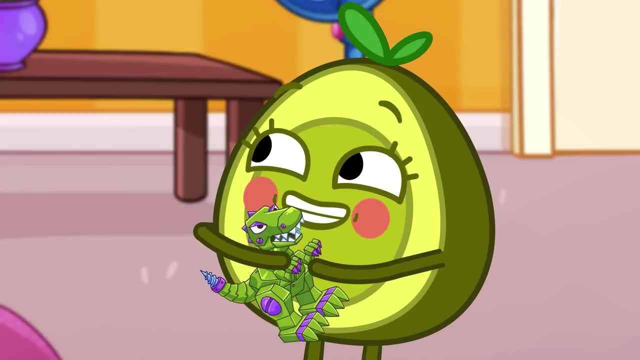 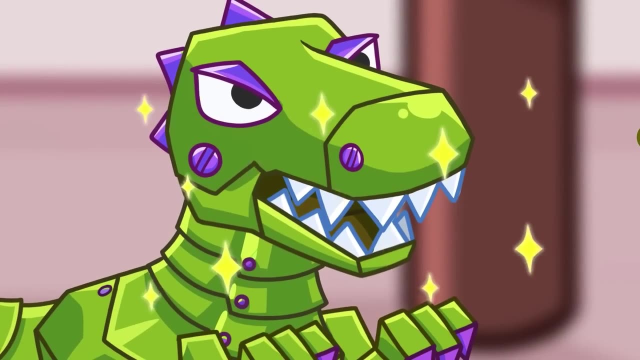 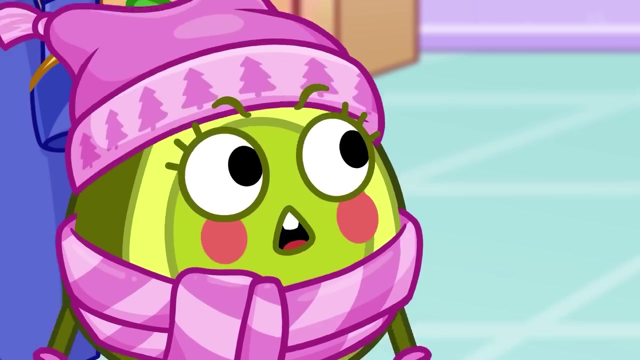 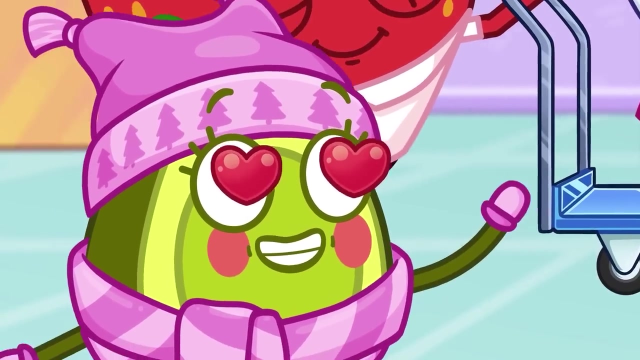 Pit is an excellent dentist. Do you remember what you have to do? Yes, Brush my teeth every day. That's right, Penny. Well done, Penny is playing dress-up, But Pit and Daddy have fallen asleep. Wake up, Pit. 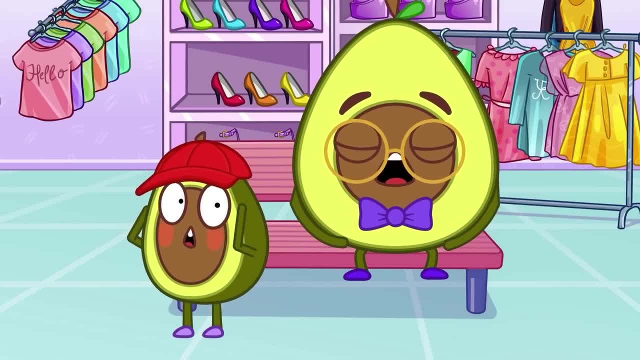 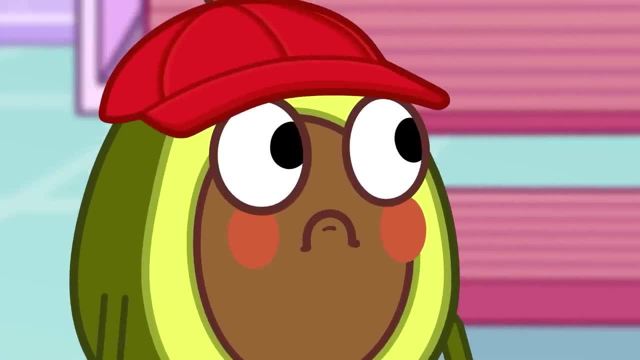 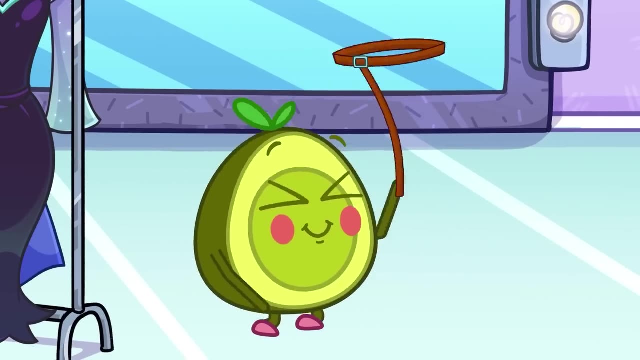 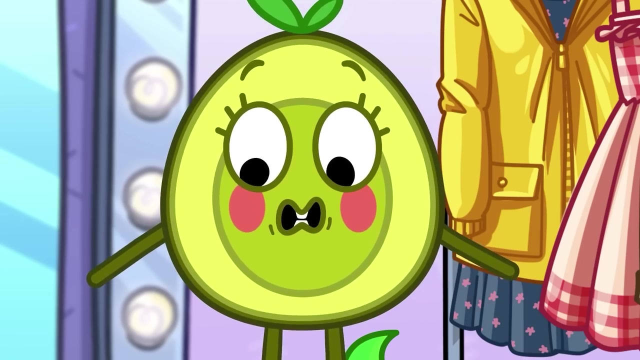 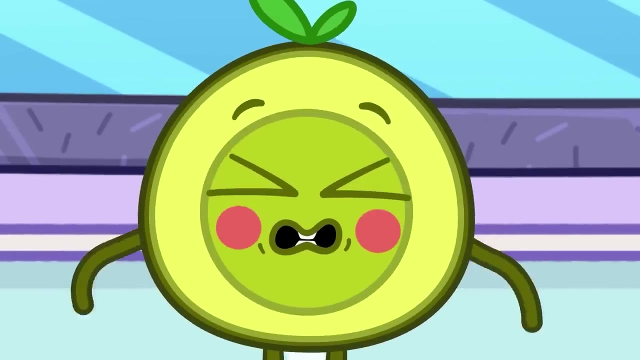 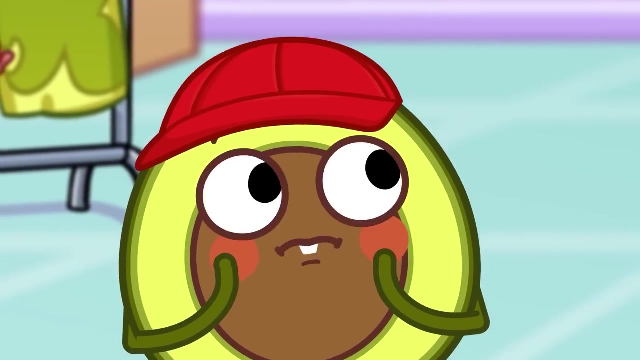 Where did Penny go? Wake up, Daddy, Dad, I don't see Penny anywhere. Penny, that's not very nice. And where is Pit and Daddy? Oh no, I'm lost. Penny, Where are you? Maybe she's behind these clothes. 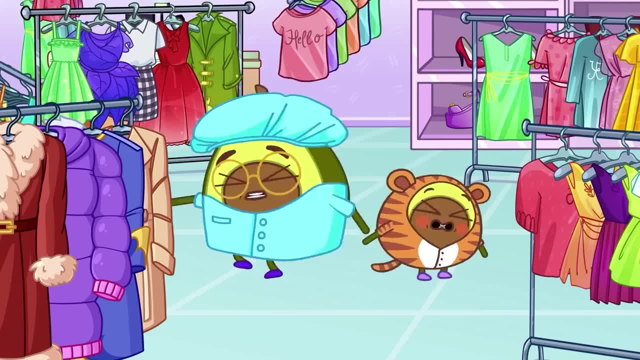 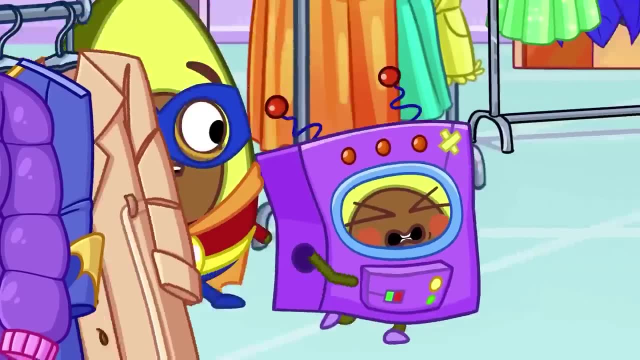 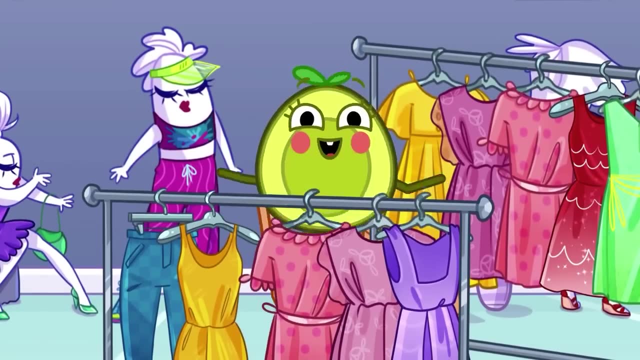 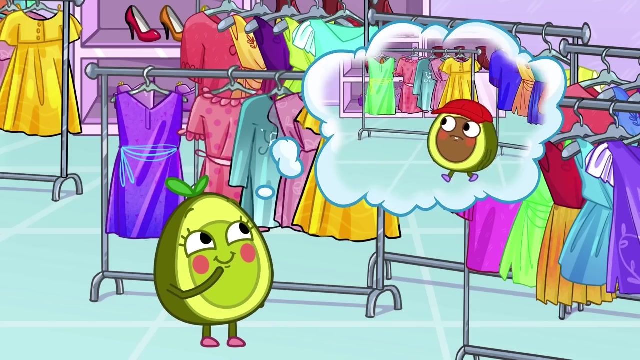 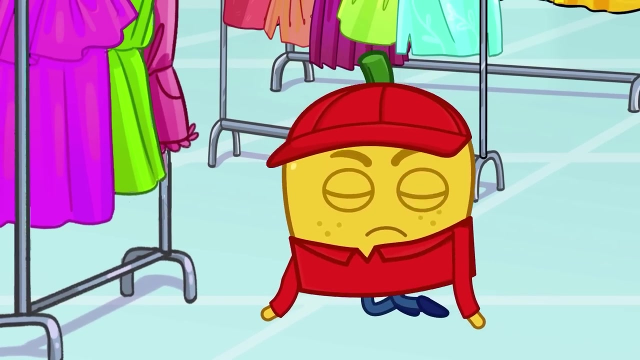 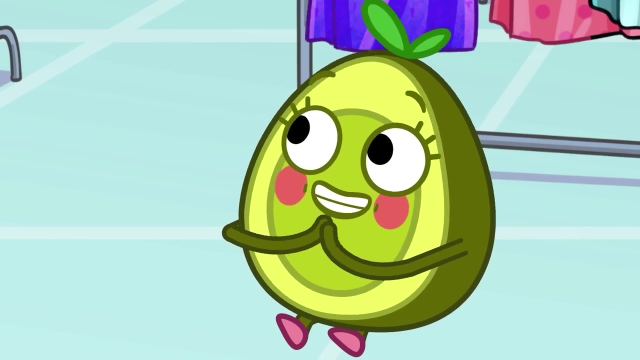 Pit and Daddy, you look silly. Oh, Not again. Watch out. Can Mommy help find Penny? Penny, that looks like Pit's hat. Oops, But that's not Pit Ugh, Oh, Maybe those are Mommy's shoes. 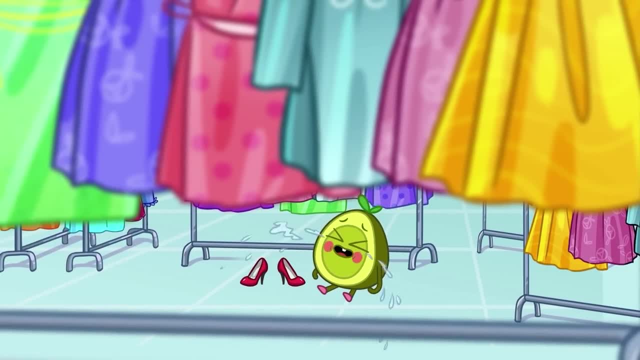 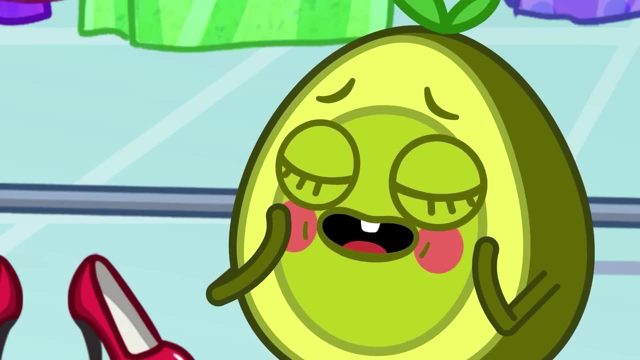 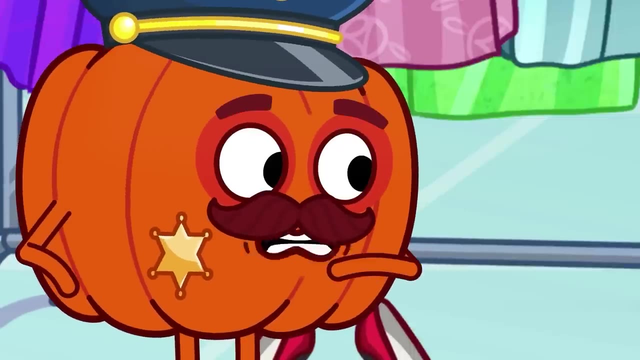 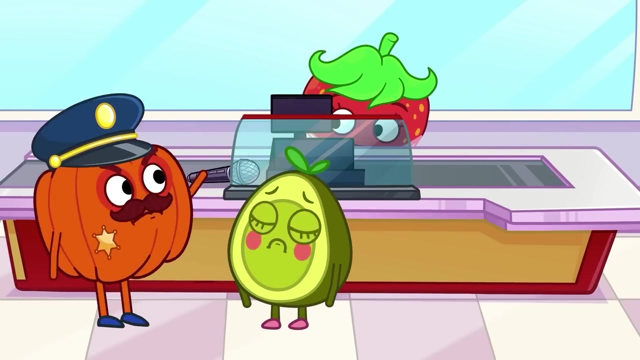 They're not Mommy's shoes. Officer Pumpkin, can you help Penny? Help me, I've got lost. Don't cry, kiddo. Help, Help, Help, Help, Help, Help. help you find your parents. attention pennies. parents, please go to counter one. 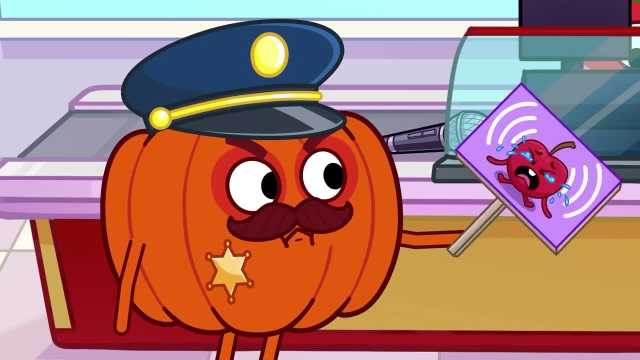 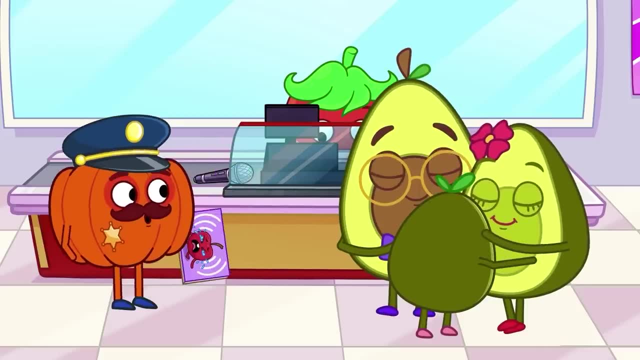 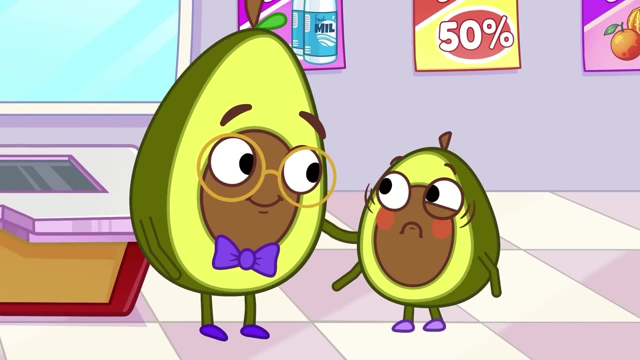 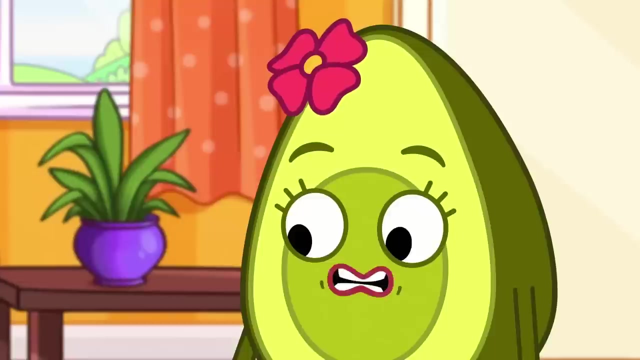 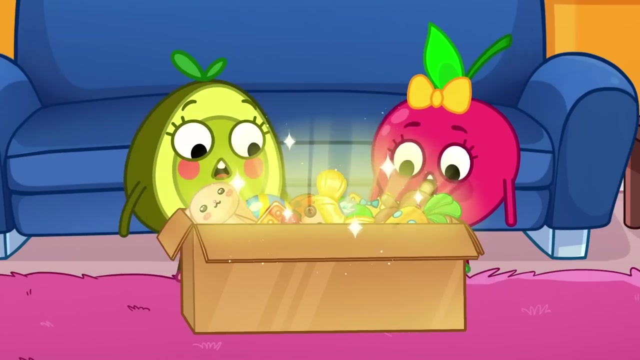 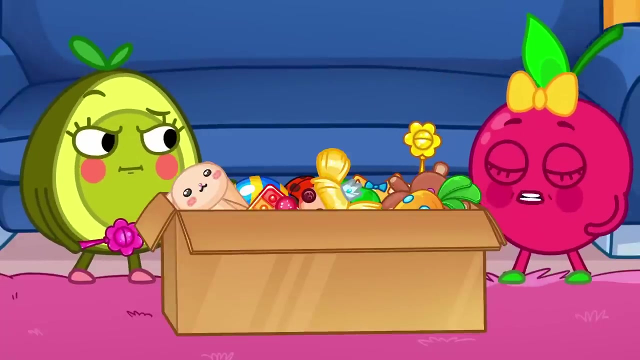 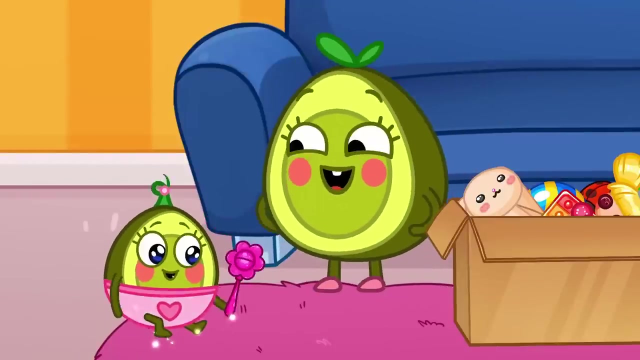 any founder family. remember if you're lost. stay where you are and call your parents. Oh, your head is stuck in a sweater. penny and cherry are playing with your sisters here, just something for your sisters to play. it's a box full of guys. cherry loves the color gold, but penny loves the color pink. I'll prove to you. 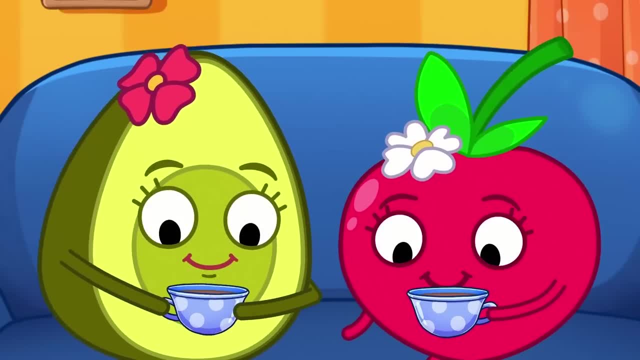 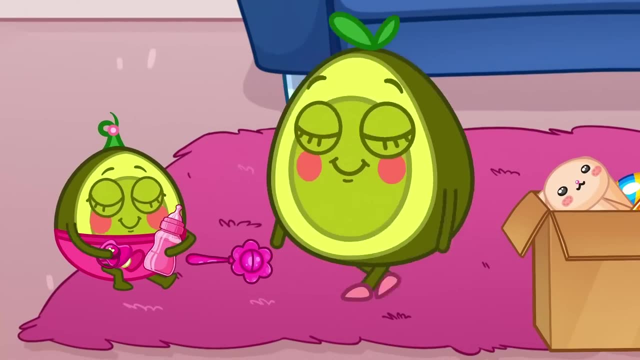 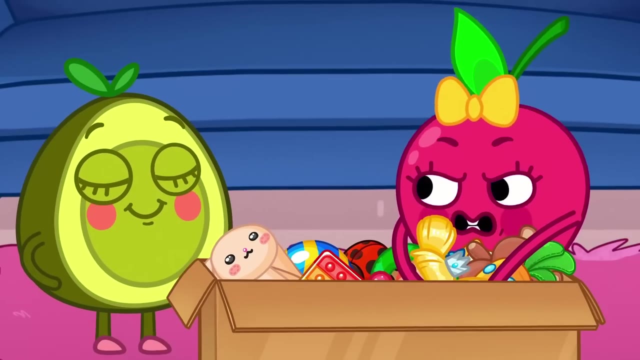 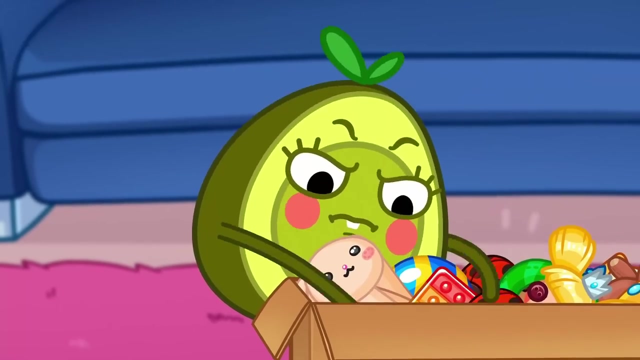 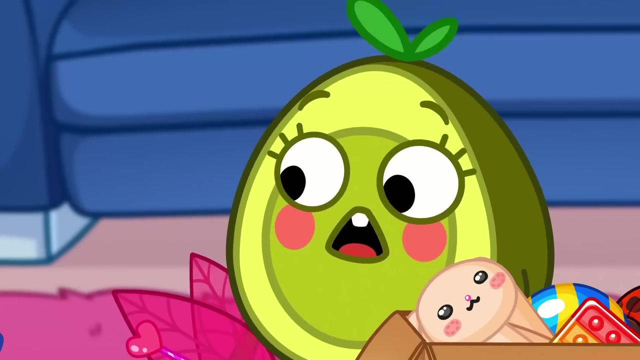 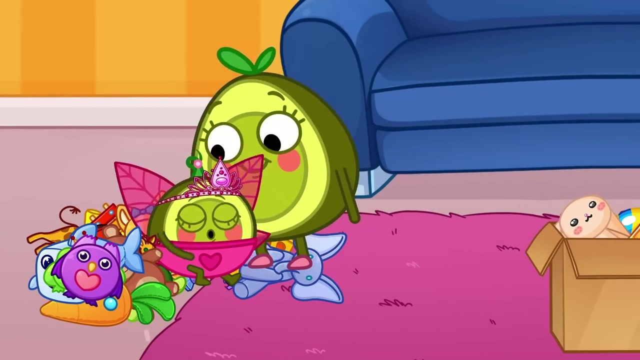 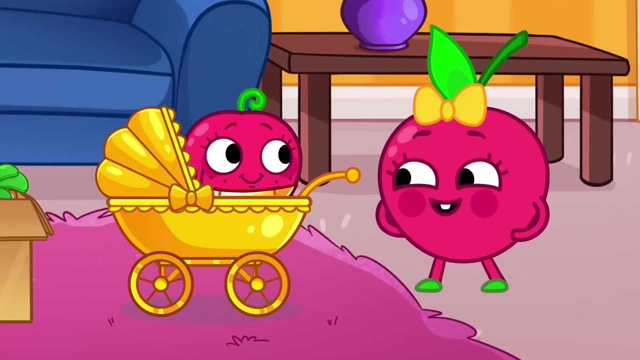 that pink is better. penny found a pink bottle and soothers cherry found a gold bottle. and soother cherry found a gold bottle. and soother, what a lovely pink tiara and wing baby is now a pink fairy. jerry has a gold stroller. oh, oh. 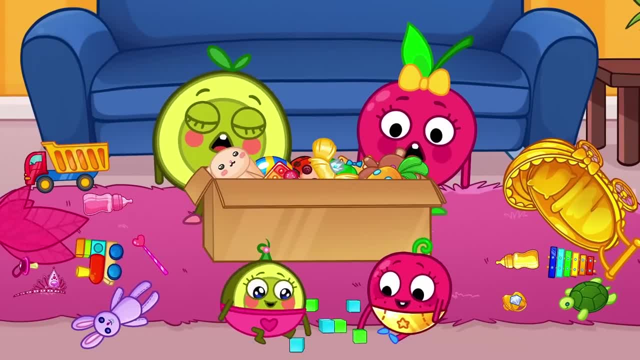 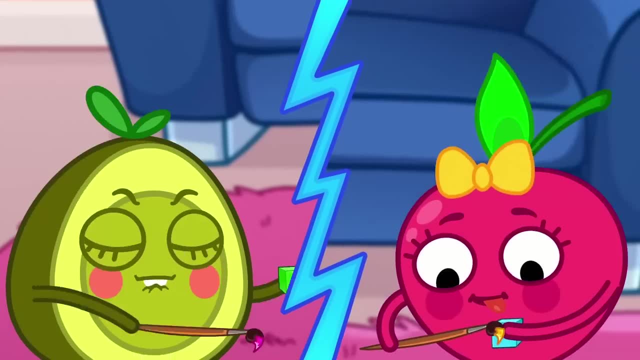 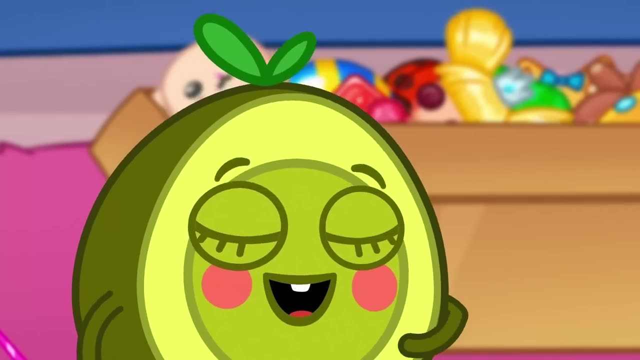 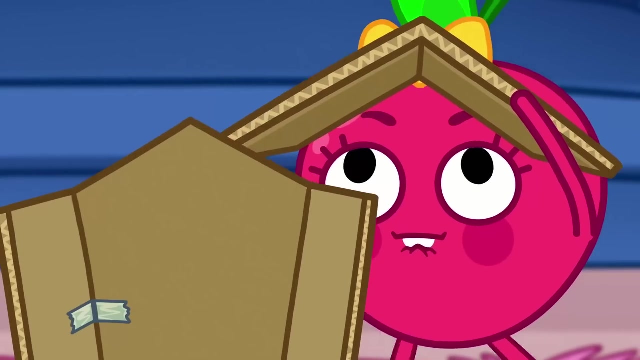 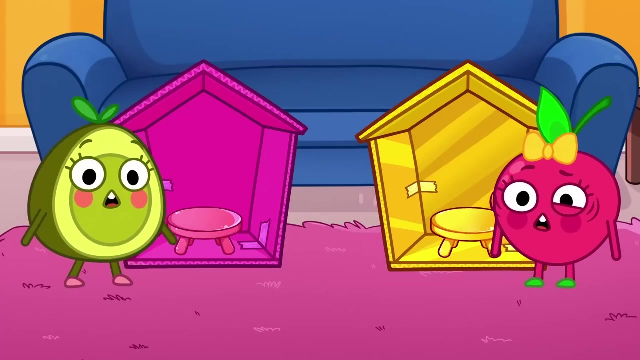 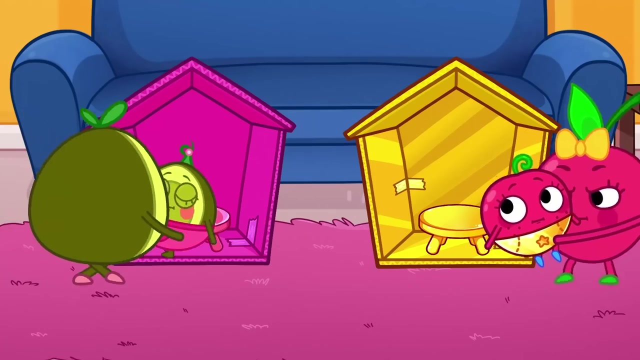 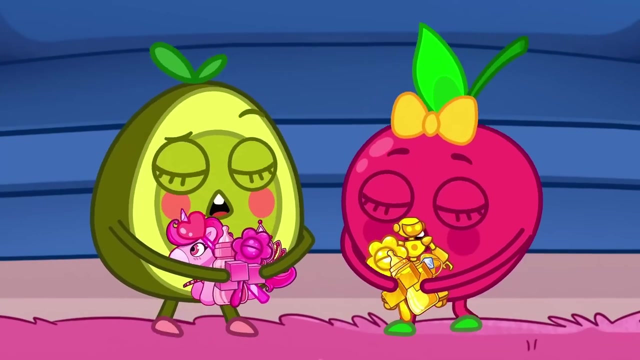 The babies are happy playing together, But Penny and Cherry aren't Gold blocks and pink blocks. What are they going to build? They made two little houses: One is pink and one is gold. But the babies really just want to play together. 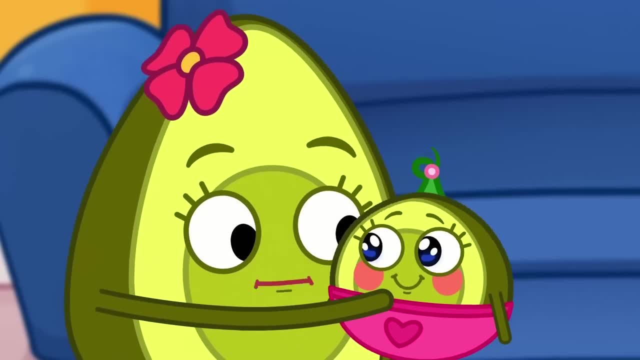 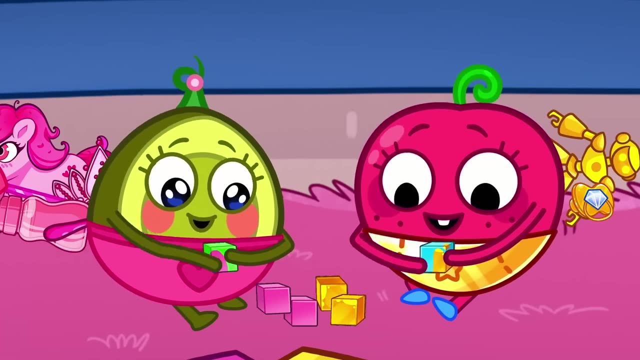 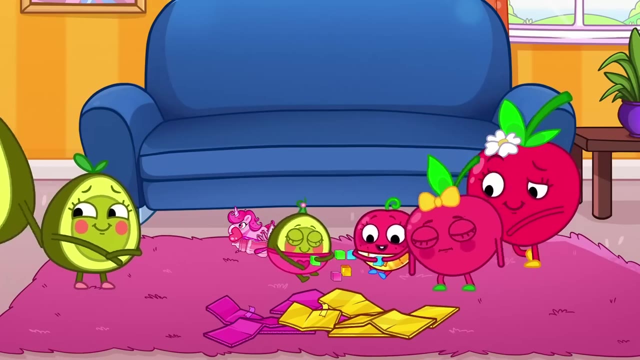 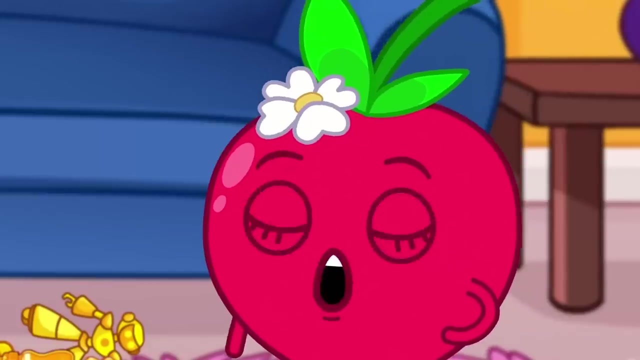 What does Mommy think? Other people will not always like the same things, as you See how happy they are. Everyone has their own interests. It's okay to be different- Mommy made cupcakes- But you can always find common interests. Pistachio is my favorite. 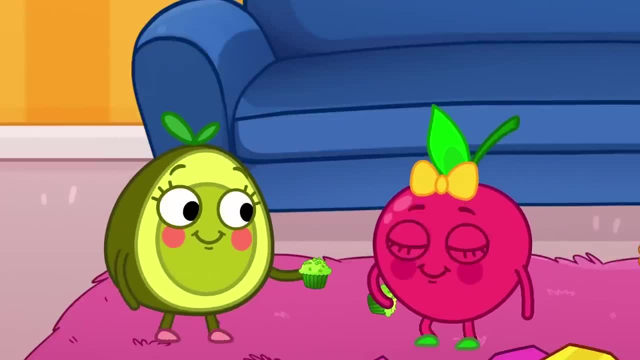 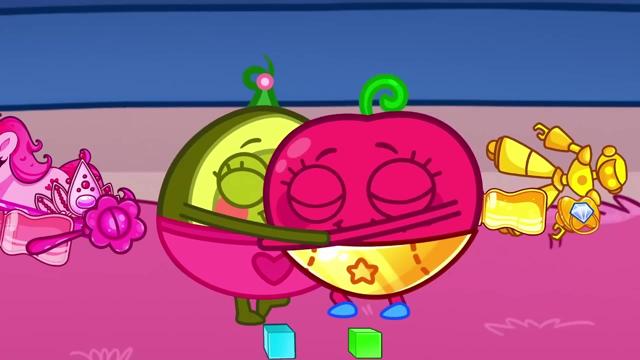 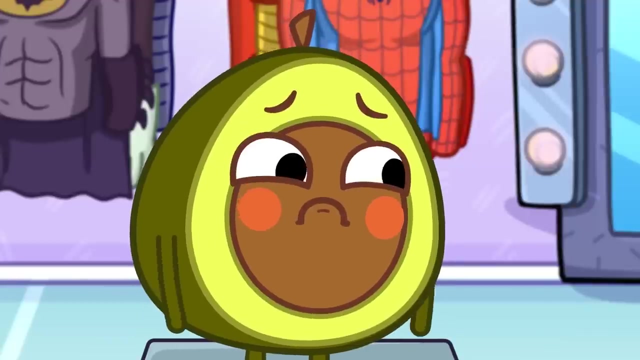 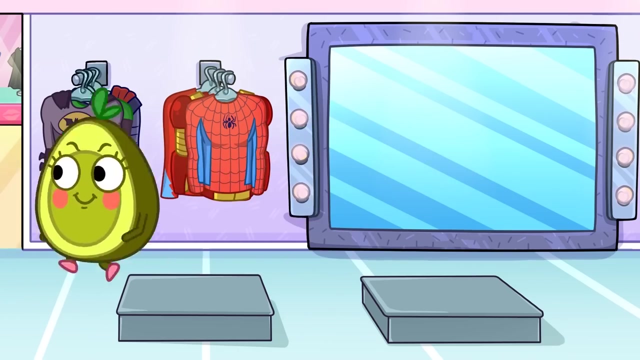 What about you, Cherry, And mine too? See, You do have something in common. Pit and Penny are trying on new clothes, But they're bored. What could make this more fun? Let's be superheroes. Who will Pit be? 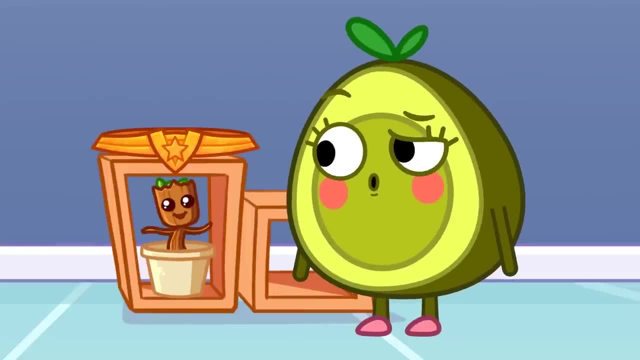 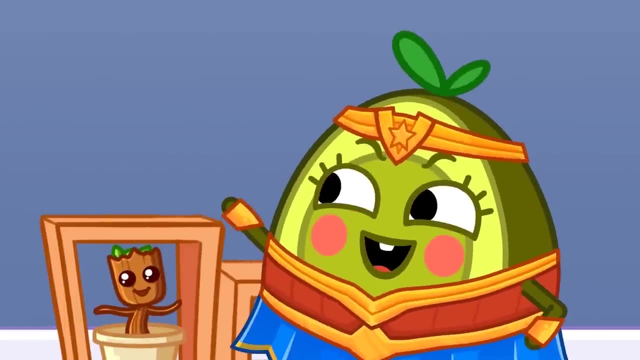 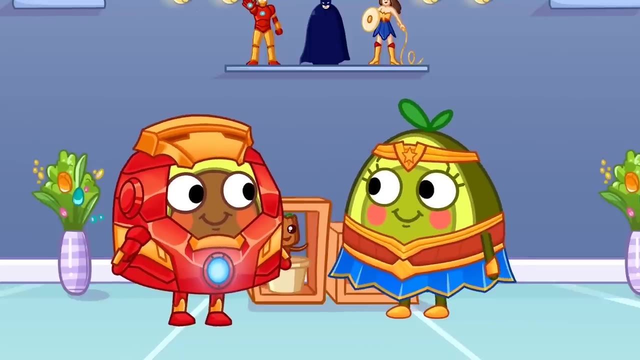 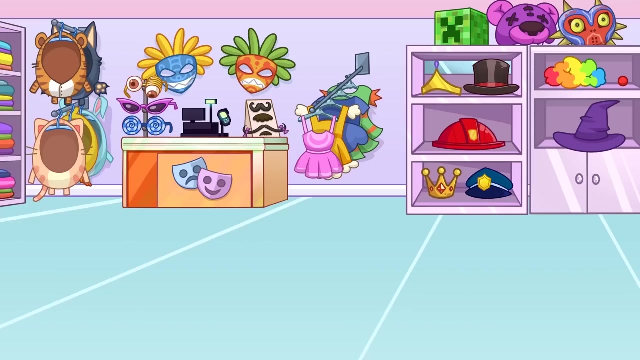 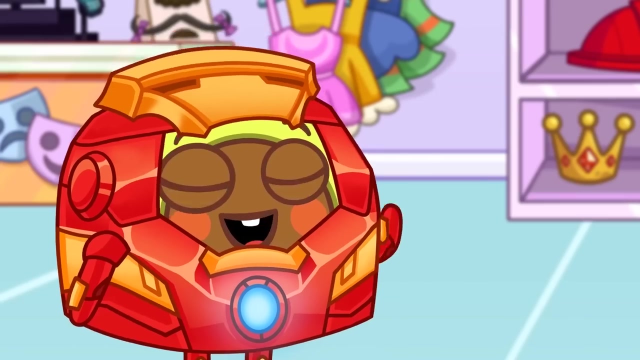 It's Iron Man, Iron Pit. And who will Penny be? It's Wonder Penny. Let's play hide and seek. One, two, three… Where will you hide Pit Pit? Maybe over there, Wow. What do you think? 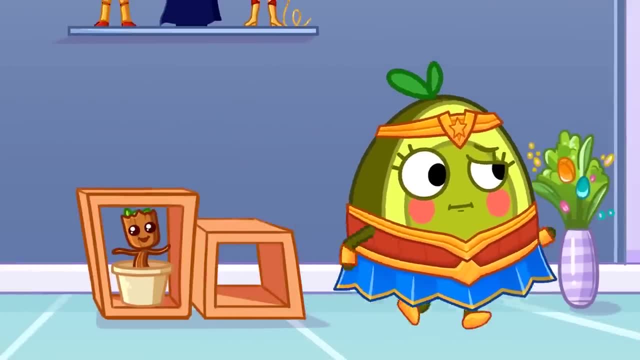 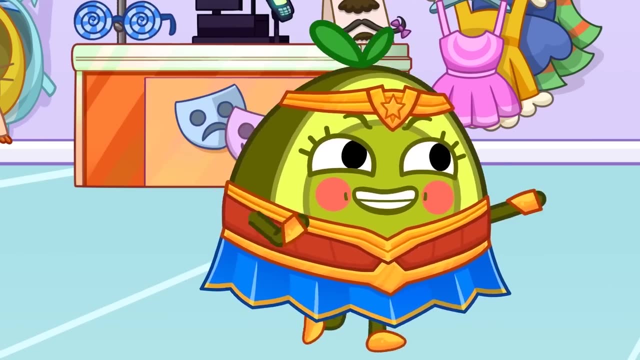 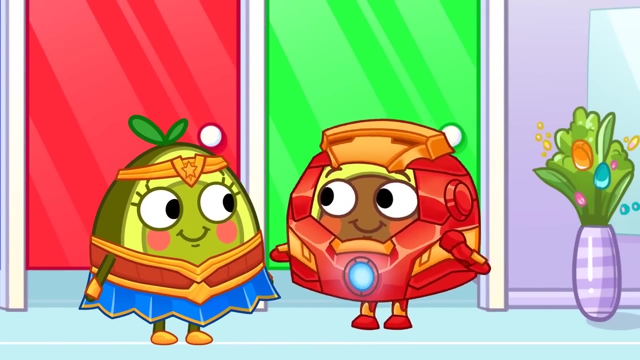 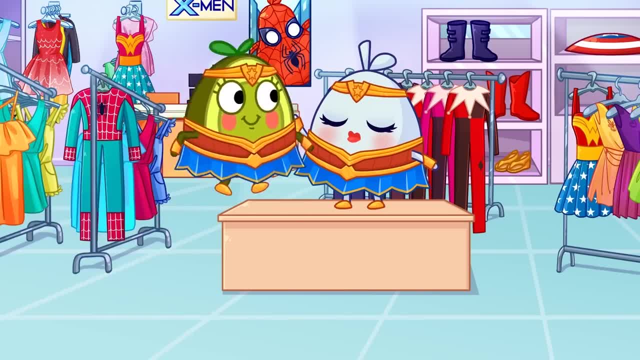 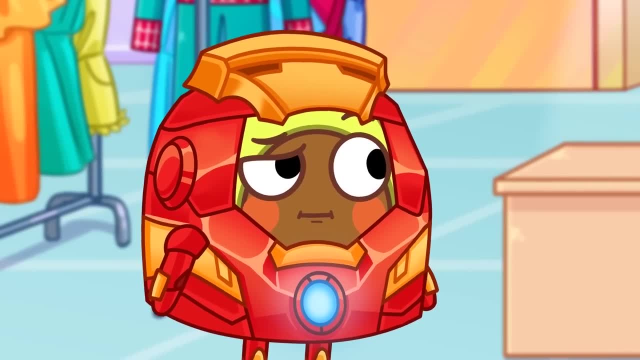 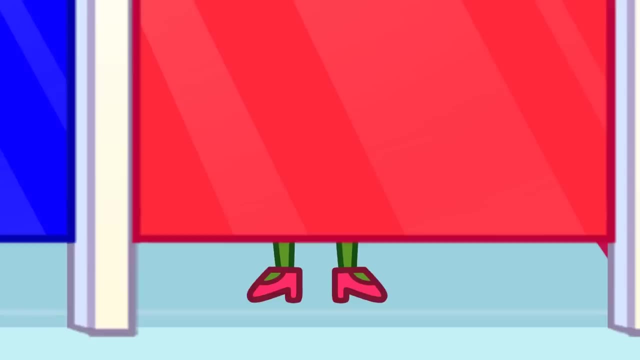 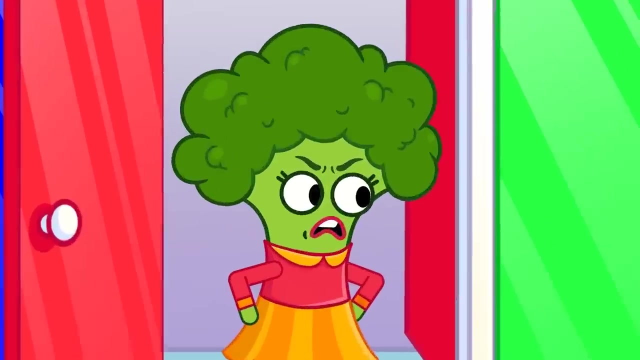 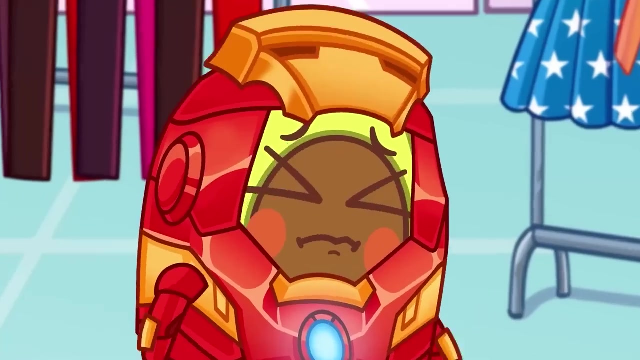 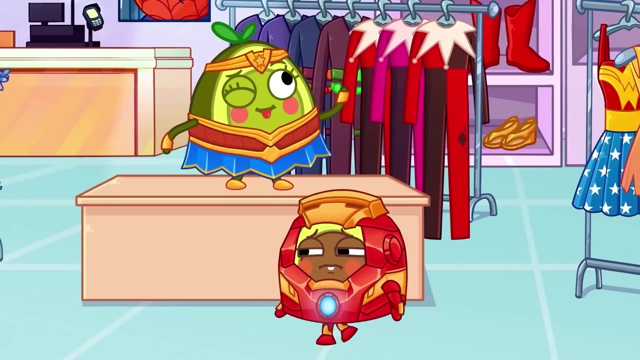 I don't know. I don't know Where will you hide Penny Pit. do you know where Penny is? No Pit, not in…. Oh, Now, where will you look? Pit? Was that? Penny Pit has an idea. 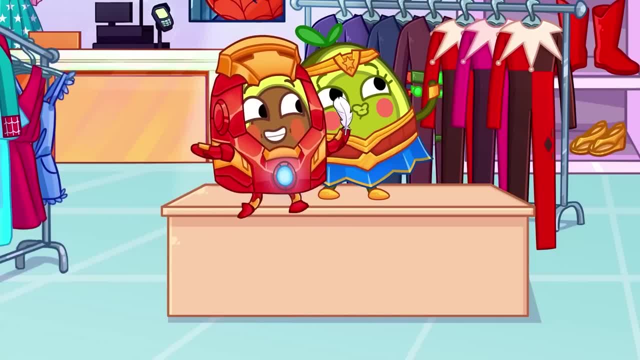 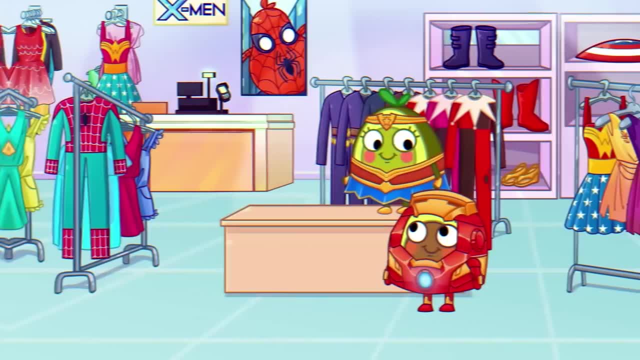 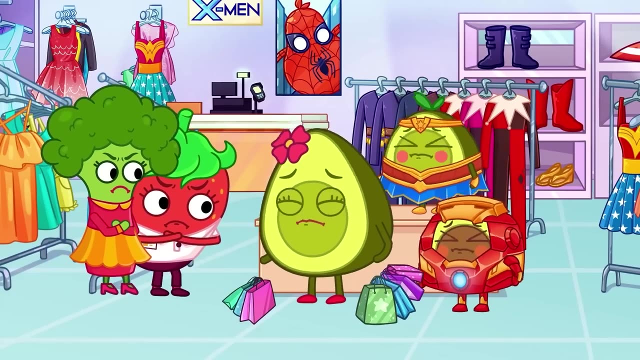 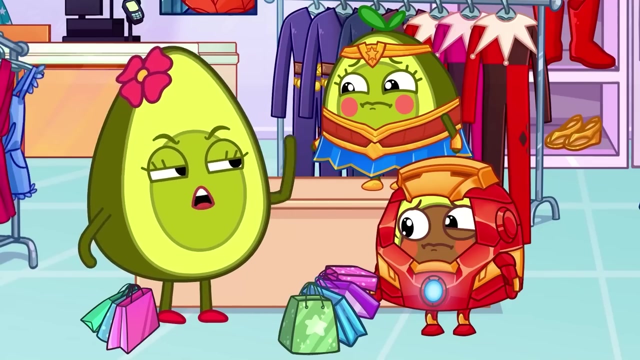 What will he do with that feather? Mommy's done shopping and it's time to go. Uh-oh, This is a clothing shop. it's not a place for games. You should learn and remember the rules of behavior. Let's clean it up. 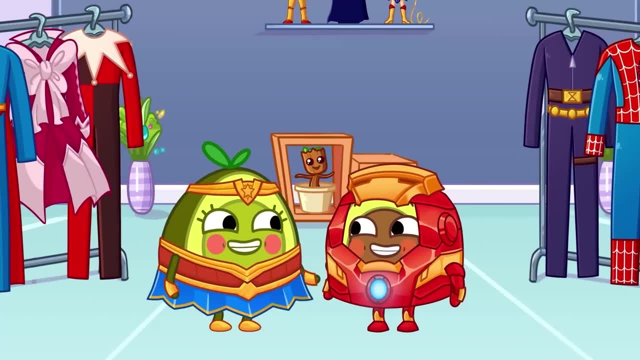 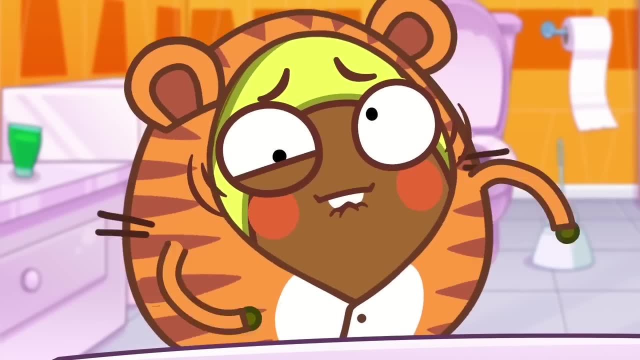 All done, Now it's time to go. Now it's time to go home. It's nighttime, where Pit and Penny live, and they are both getting ready for bed, But Pit doesn't want to brush his teeth. That's why his breath is stinky. 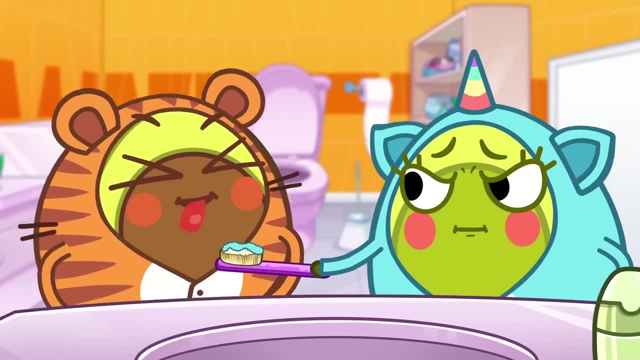 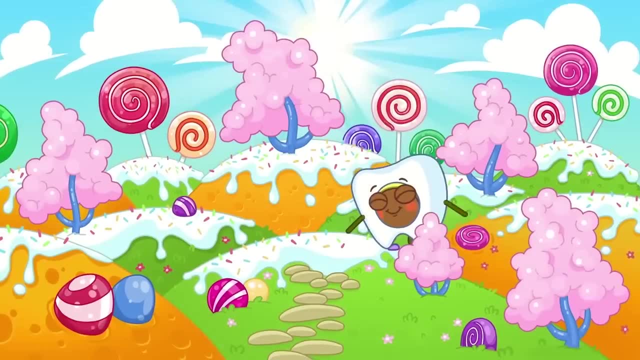 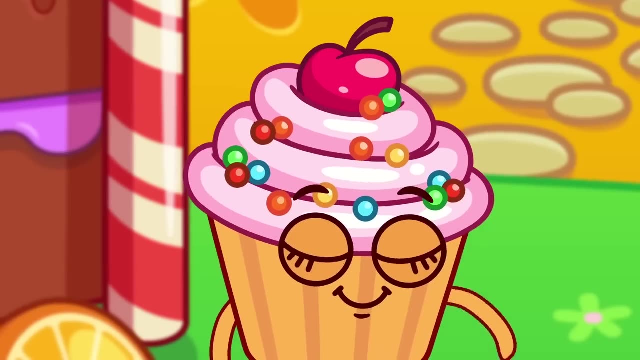 Pee-yew. Come on, Pit, brush your teeth. Pit and Penny are sound asleep and Pit is having a dream. In the dream he's a tooth and he's surrounded by candy. Three new friends want to play Cupcake, lollipop and chocolate. 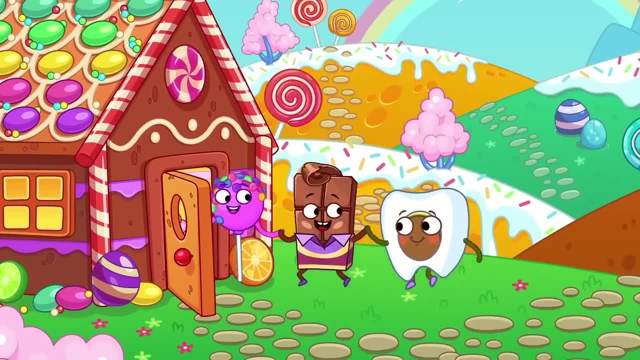 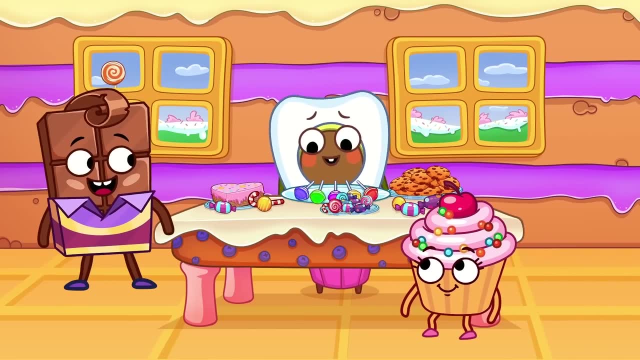 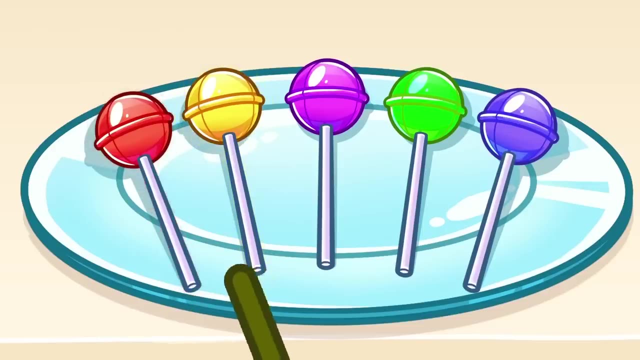 Pit is very happy to meet them. Look at all those sweets and treats. Pit wants to eat them all. Lollies are his favorite. What are the colors Pit? Red, Yellow, Pink, Green, And he eats them all in one big gulp. 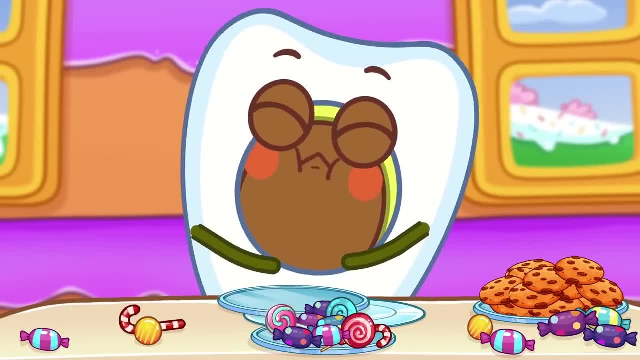 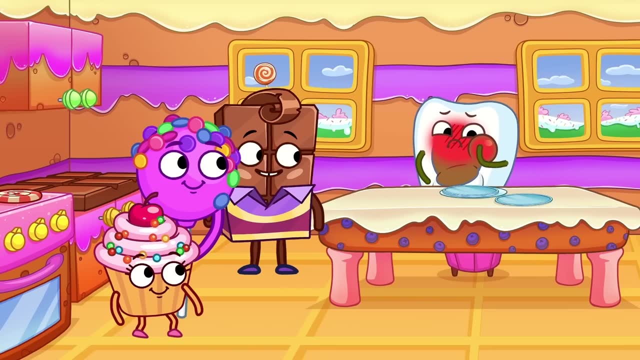 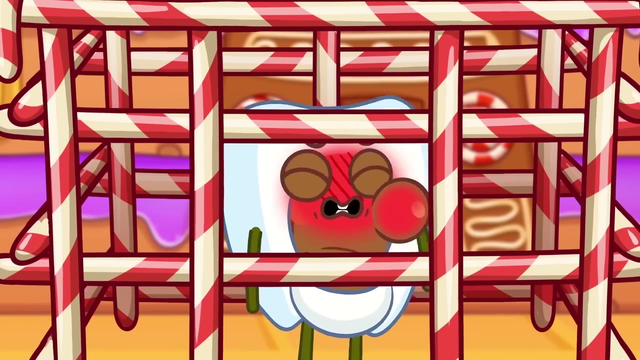 You better be careful, Pit. Too many sweets are not good for you. Oh Pit. Now Pit has a toothache And his new friends think it's funny. They even trap him in a candy cane cage. Don't cry, little Pit. 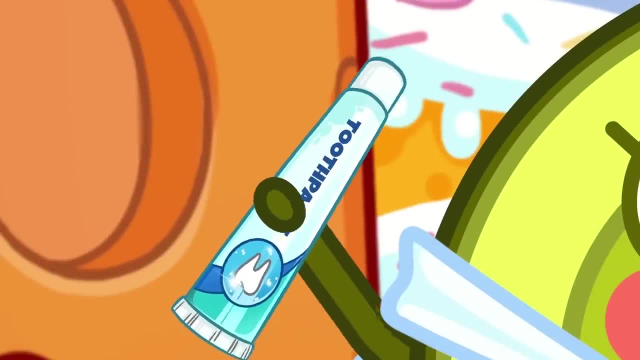 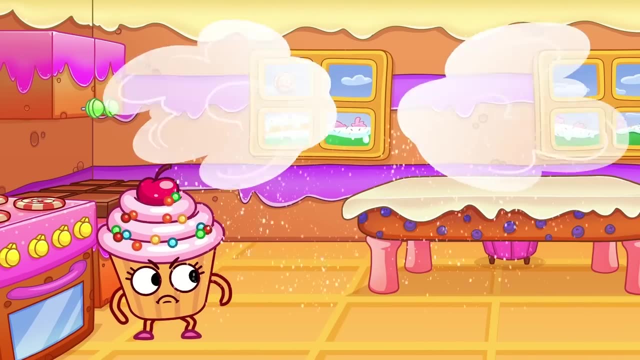 Someone's coming to save you. It's Penny, And she brought the toothpaste. Go get him Penny. Bye-bye chocolate, So long, lollipop, See you later. Cupcake. Penny even gets rid of Pit's toothache. 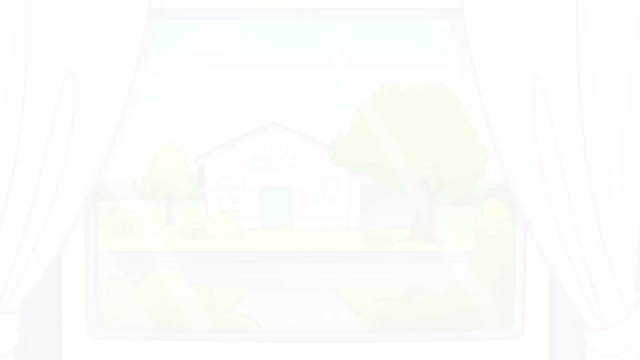 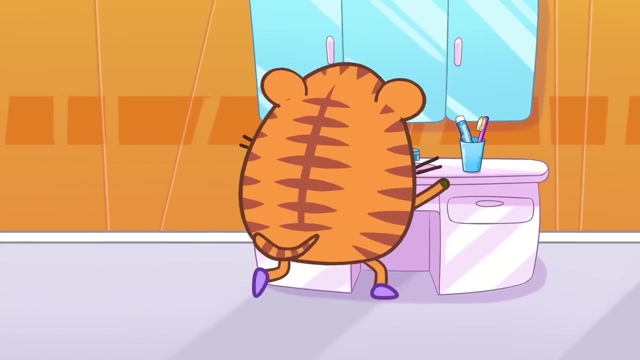 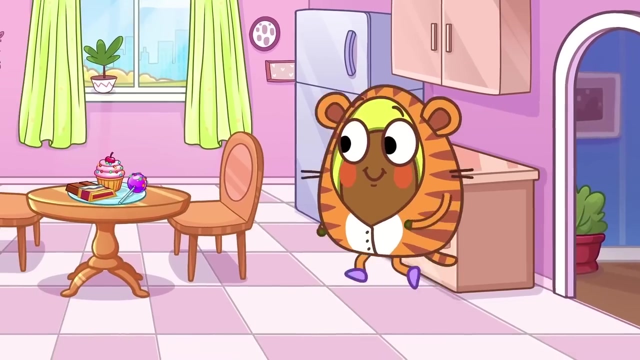 Pit is free And he's so happy to see his sister. It is now morning where Pit and Penny live. Good morning Pit. But where is he going? Pit is brushing his teeth. Well done, But what's on the table? 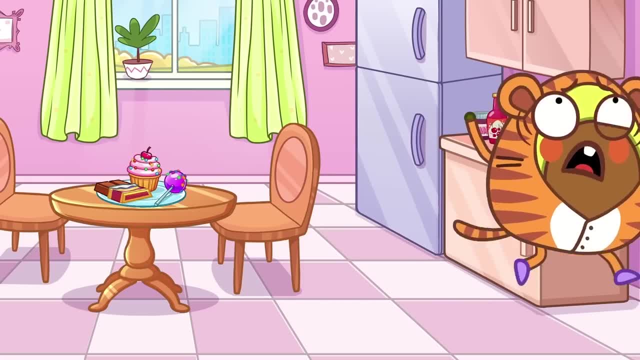 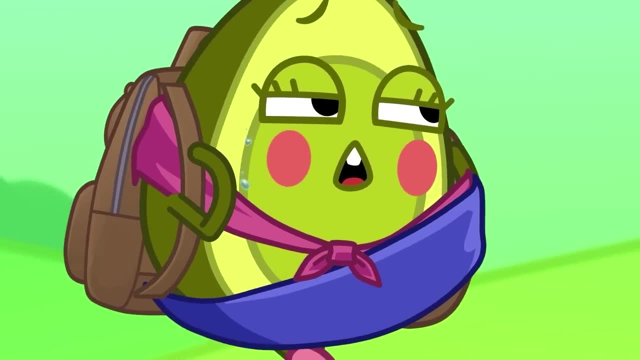 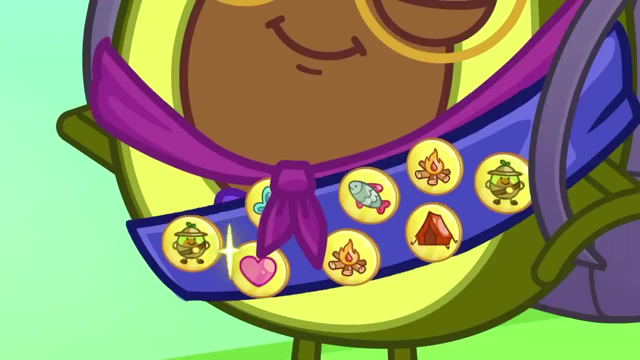 Uh-oh, It's the candy from the dream. Pit and Penny are hiking a big hill. Phew, They made it. Daddy is already there. Look at all his scalp medals. They want some too. Don't worry kids. 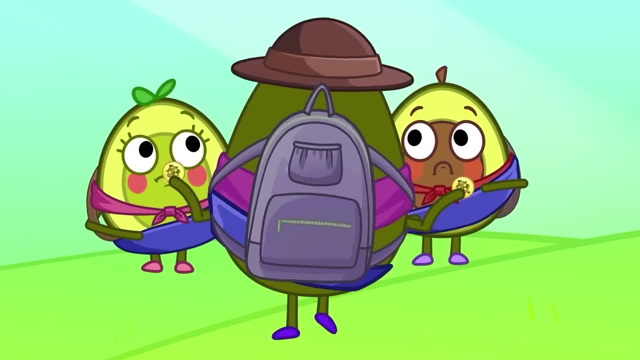 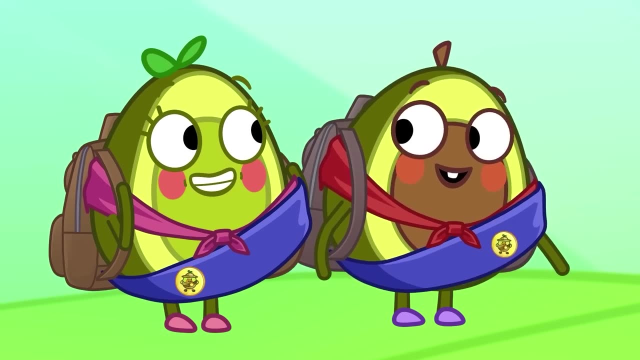 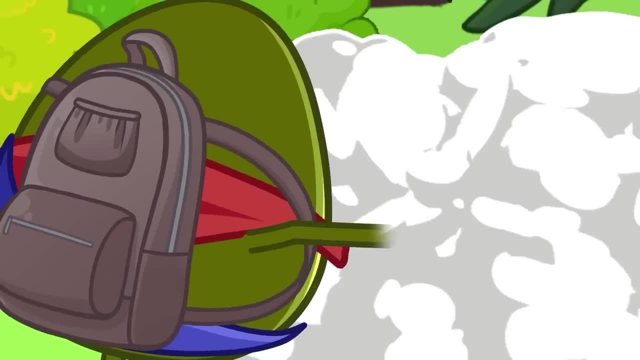 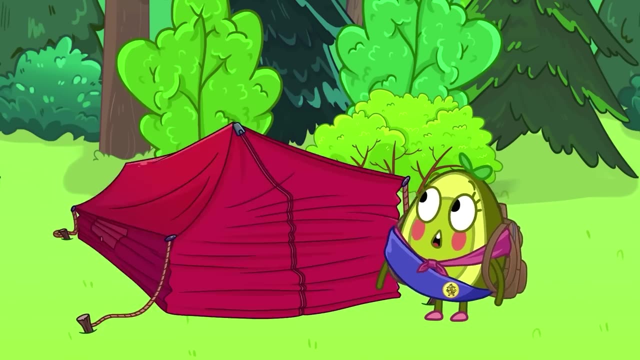 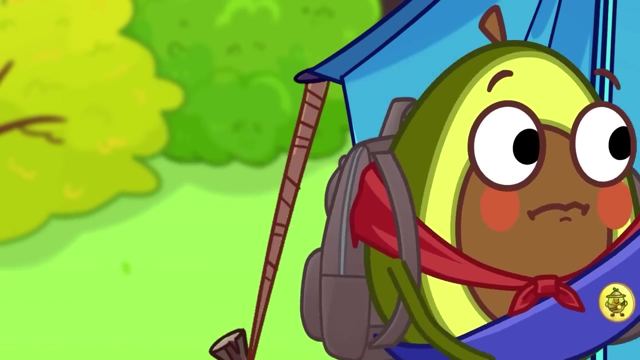 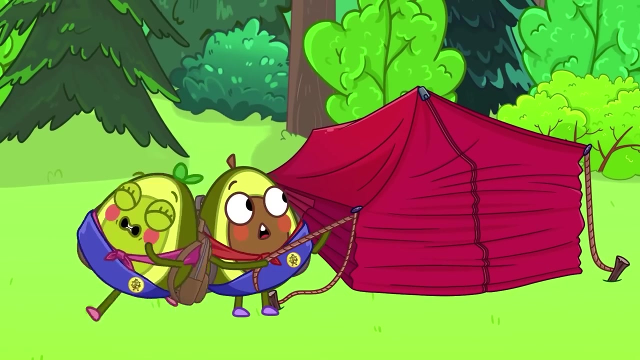 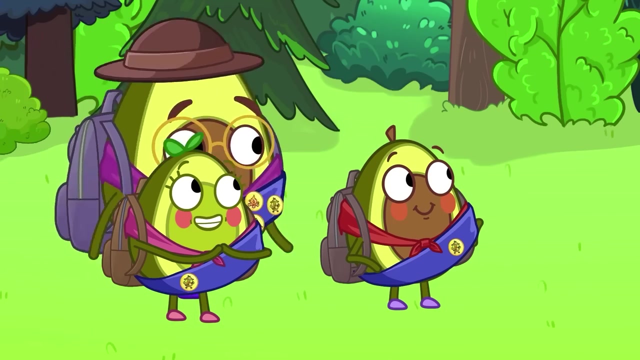 He-he-he, He-he-he. Now let's set up a tent. Good job, Pit. You almost got it, Penny. Maybe Pit can help. You did it Together. Together, You both get a tent medal. Da-da-da-da-da-da. 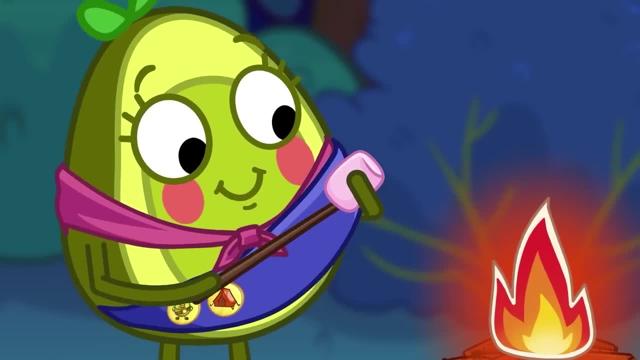 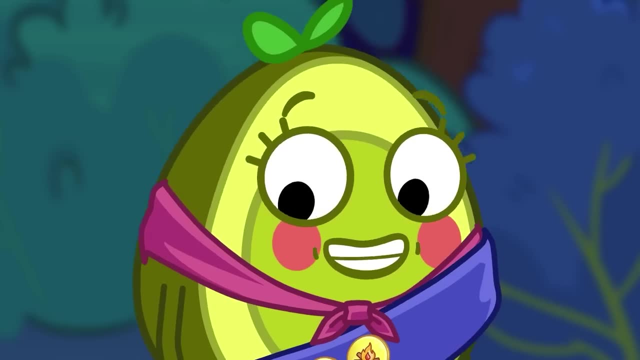 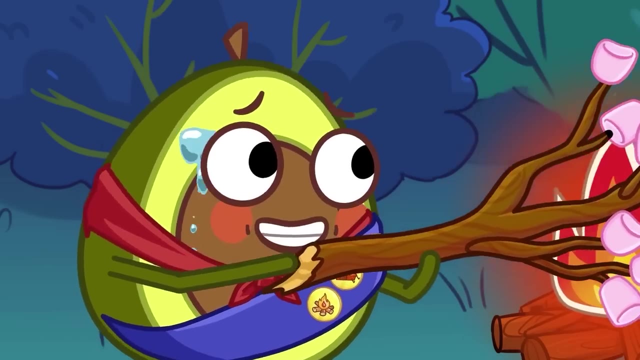 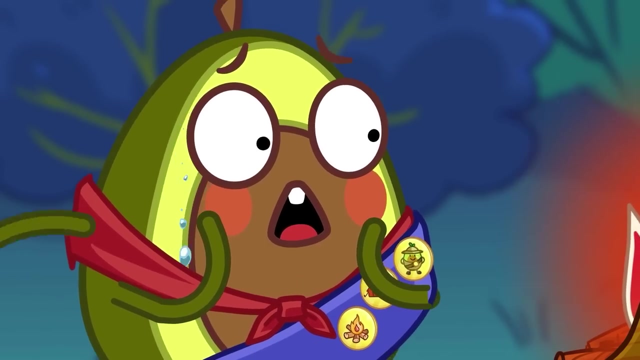 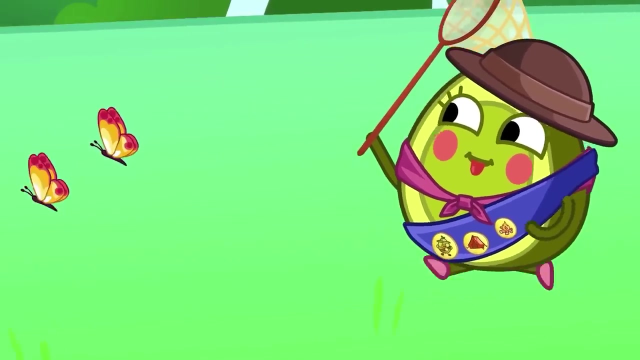 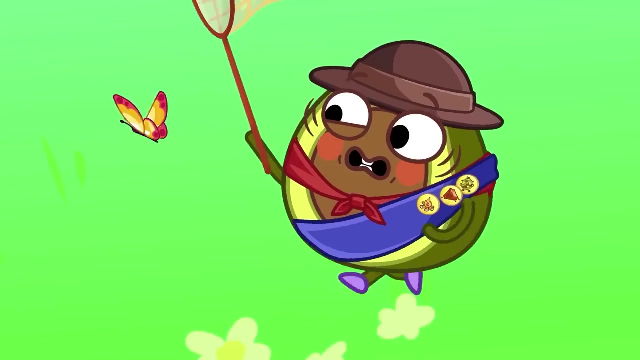 Campfires are perfect for roasting marshmallows. Good job, Penny. Pit would like a medal too. That branch was too heavy, But Penny is here to help. Wow, What pretty butterflies Penny caught. one Pit isn't as lucky. 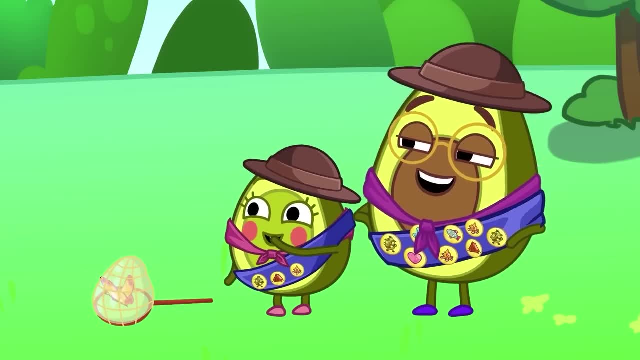 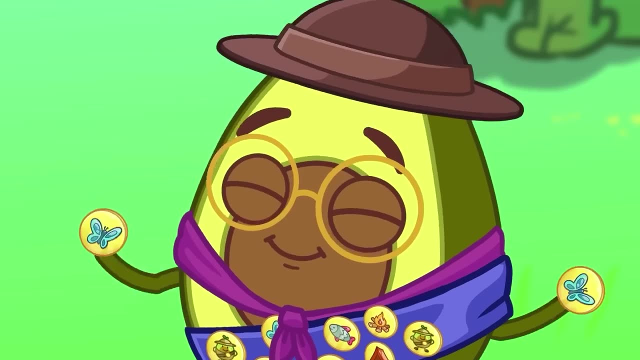 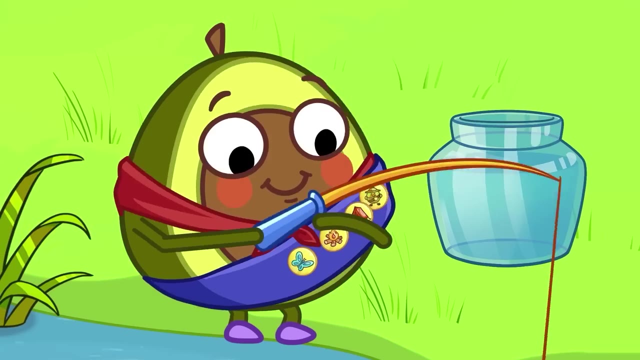 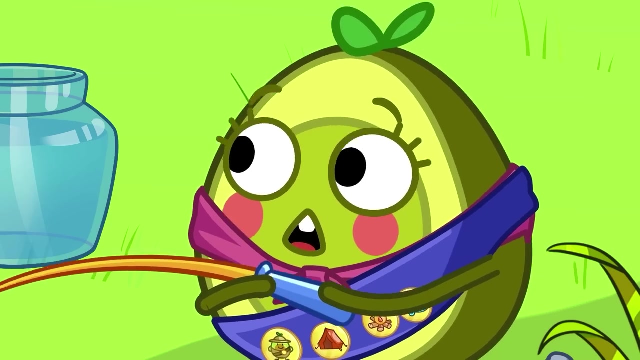 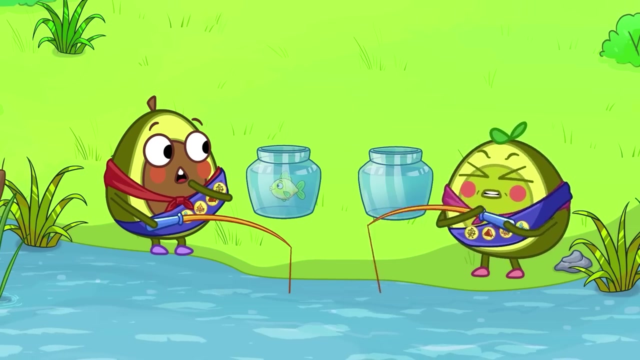 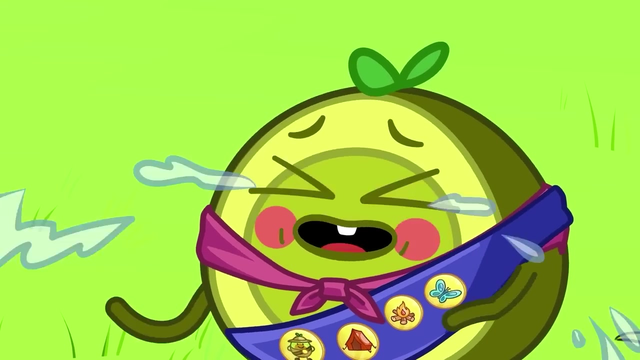 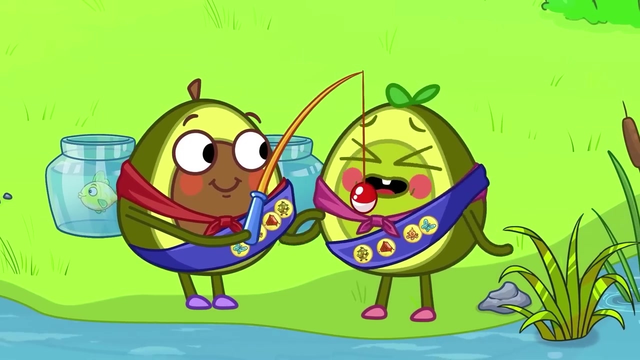 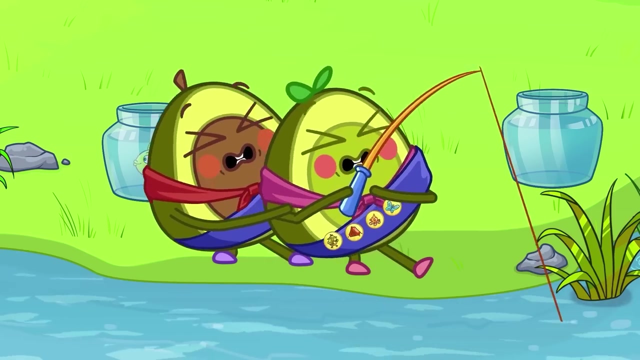 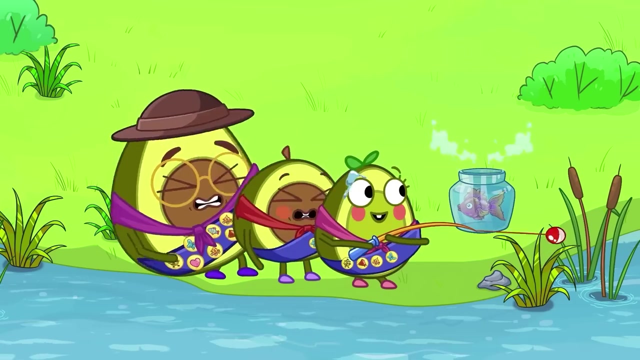 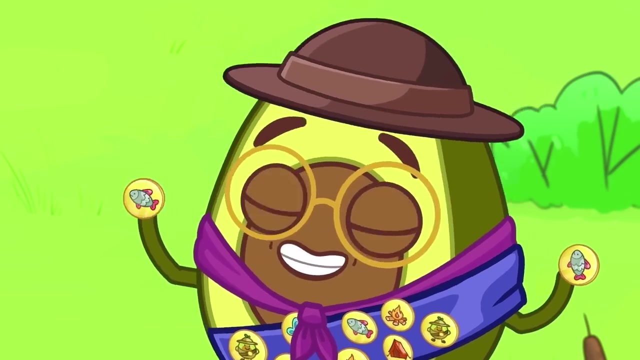 Look, Pit, They came to you Bye-bye butterfly And you each get a butterfly medal. Pit caught a fish, But Penny lost her fishing rod. Help your sister, Pit. Penny caught a big fish. Yay, More medals. 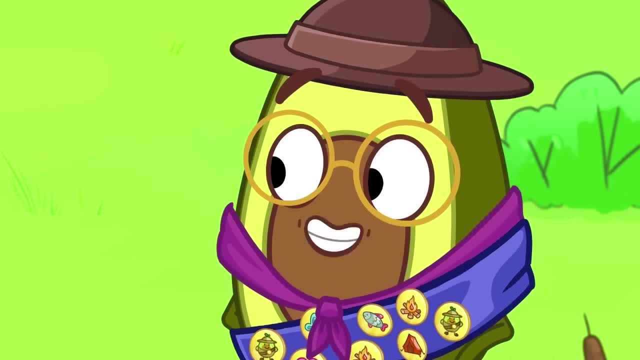 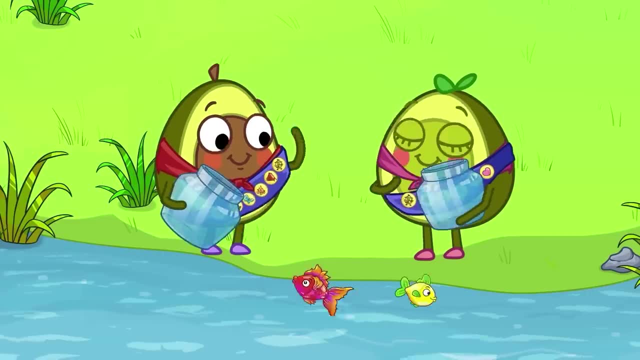 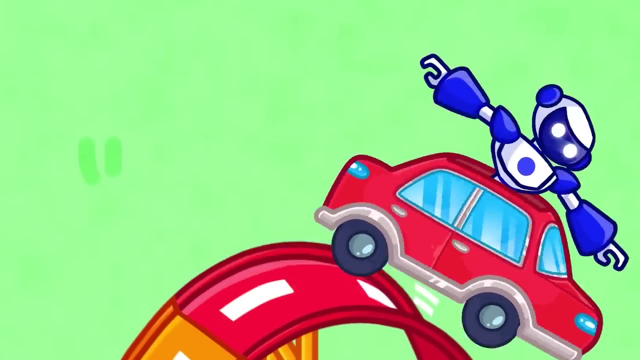 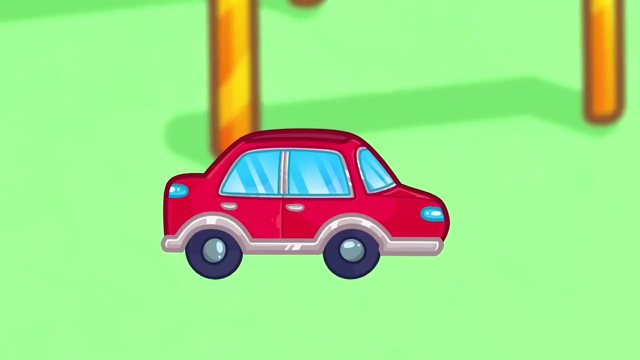 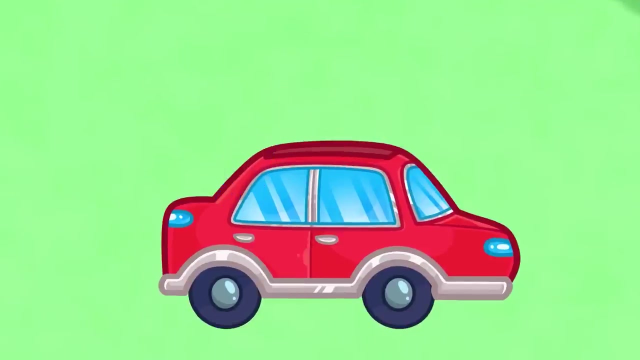 What are those medals for? And this is for friendship. Time to let the fish go. Bye, Pit, Bye. Penny Blueberry's playing in the park. Something is missing. Oh, The robot is gone. Oh, Oh, no, I've lost my robot. 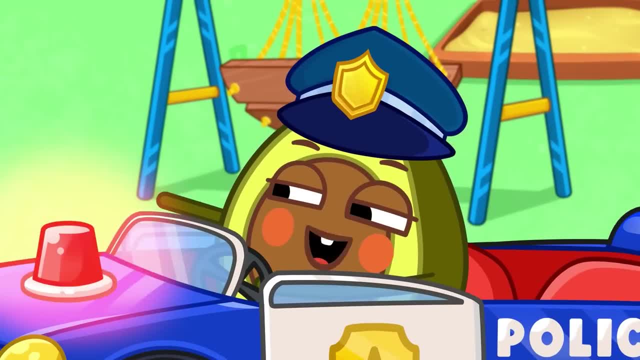 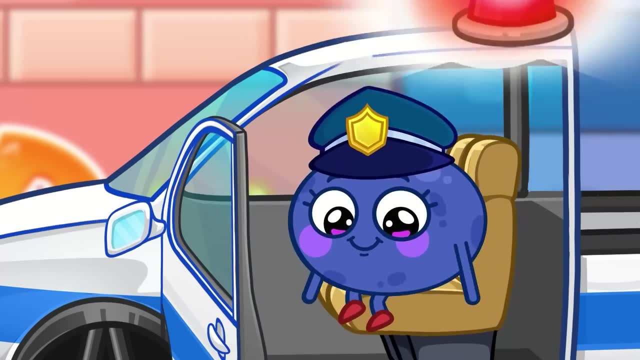 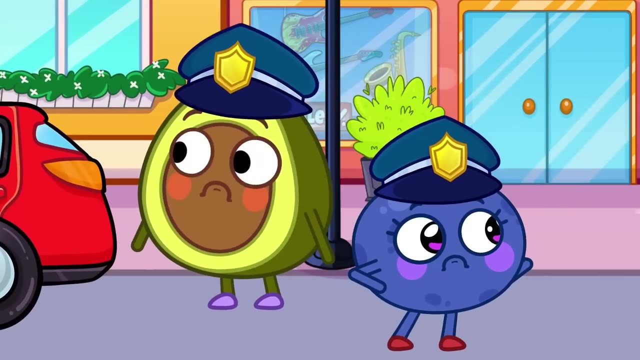 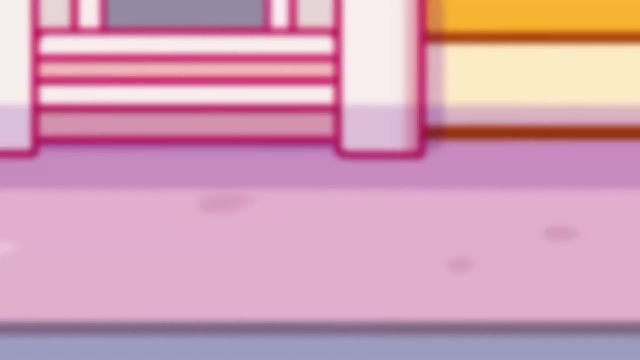 Officer Pit, can you help? If something is lost, the police will find it. Where do you think it is? Did it fall into the manhole? Let's go, Blueberry, It's a treasure chest. Oh no, Oh no. 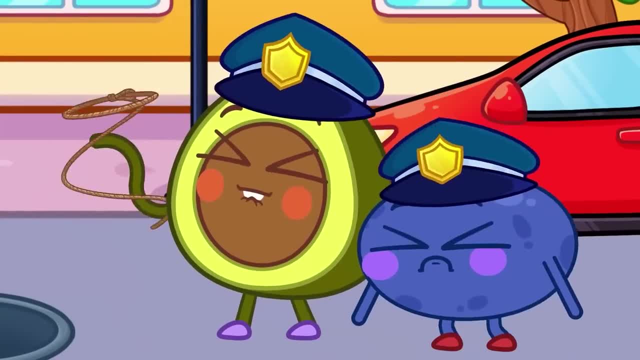 Oh no, Ah, Oh, Oh no, Oh no, Uh-oh, Ah, Oh no, Ah, Huh, Uh-oh, Uh-oh. What Uh-oh, Ah, Oh, Uh-oh. 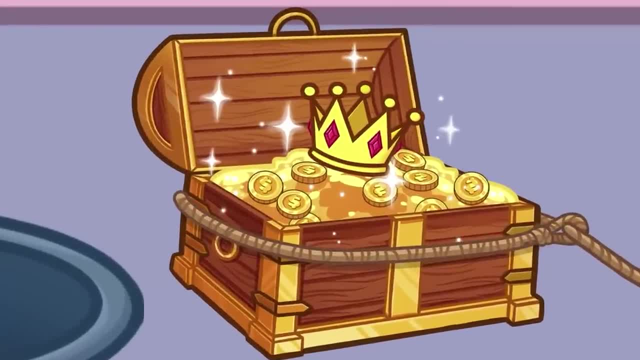 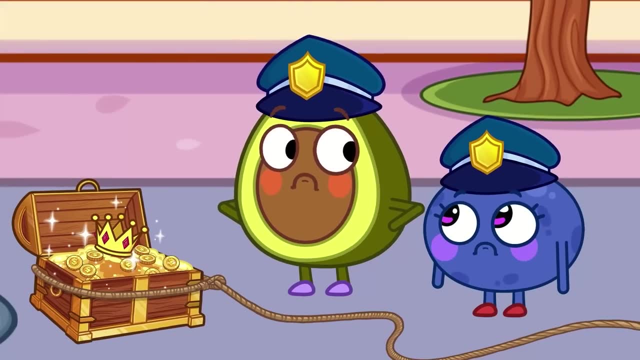 Oh, Uh-oh, Oh, Uh-oh, Ah, Ah, It's a treasure chest filled with gold. Whoa Oh, It's not a robot. It's not a robot. Try looking through your binoculars, Blueberry. 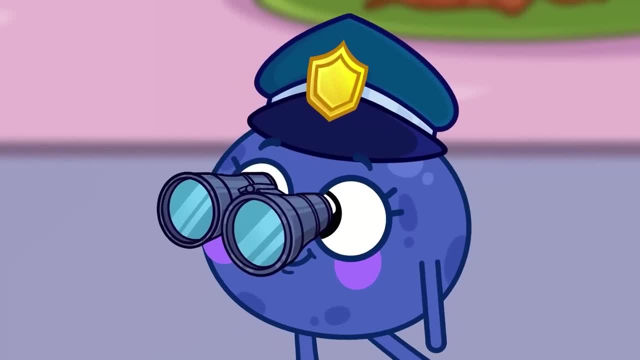 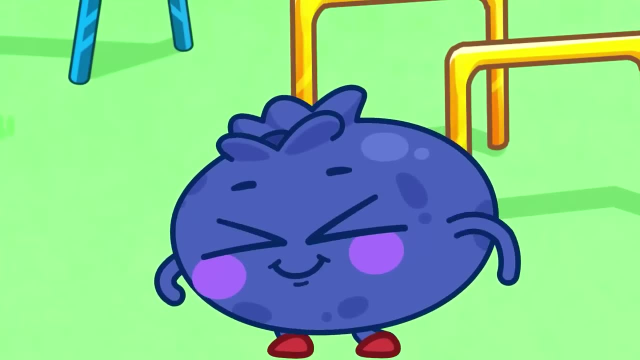 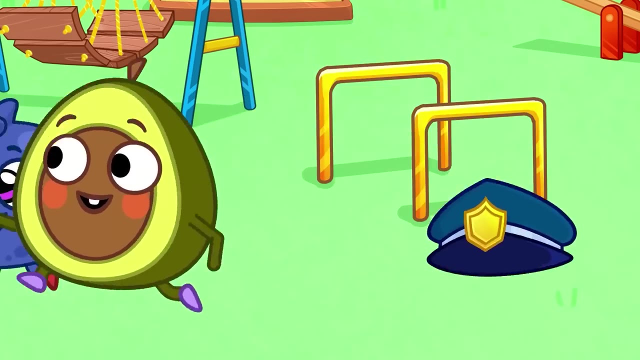 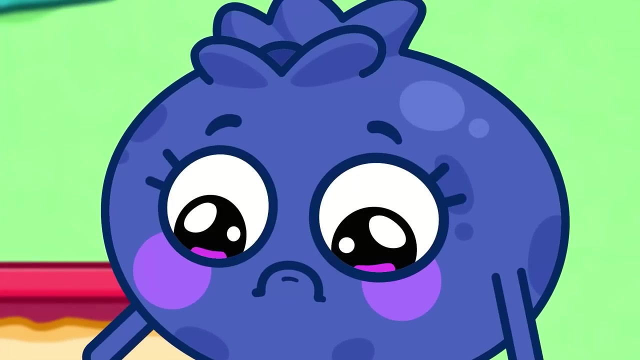 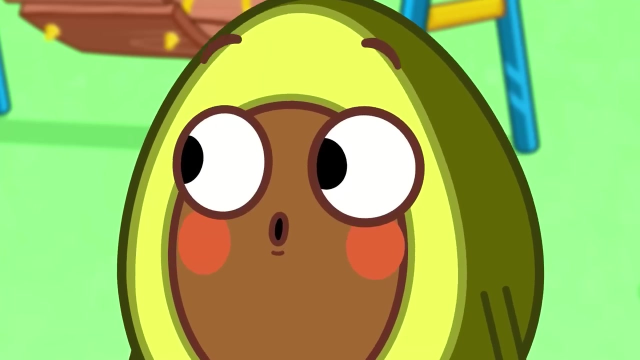 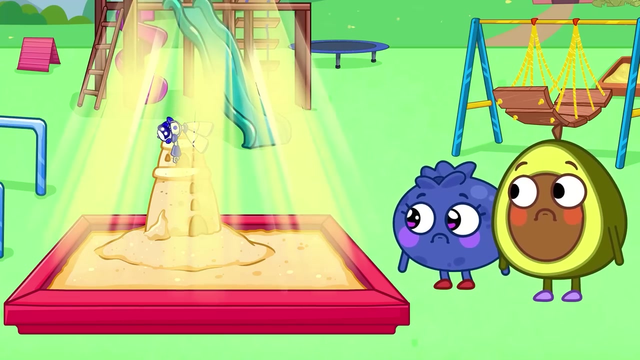 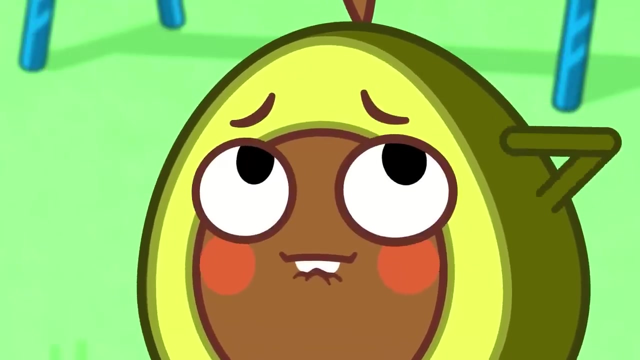 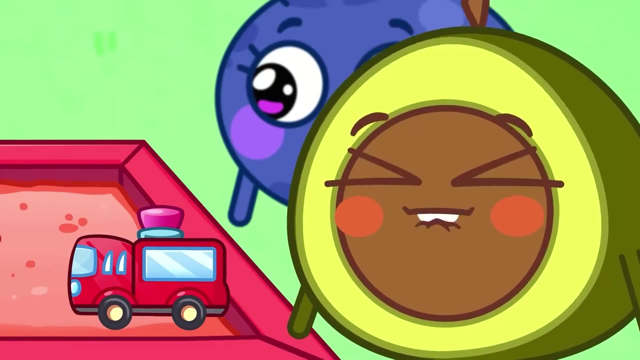 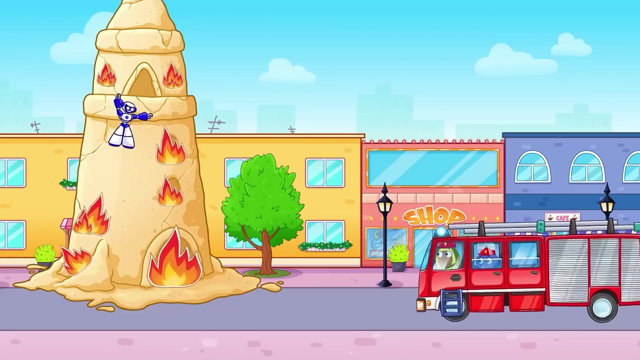 No, Uh-oh, I found the robot. It's in the sandbox. But be careful, The sand is hot. Sand often gets hot on sunny days. You need another plan. Pit Firefighters will save us from the fire Time to put the fire out. 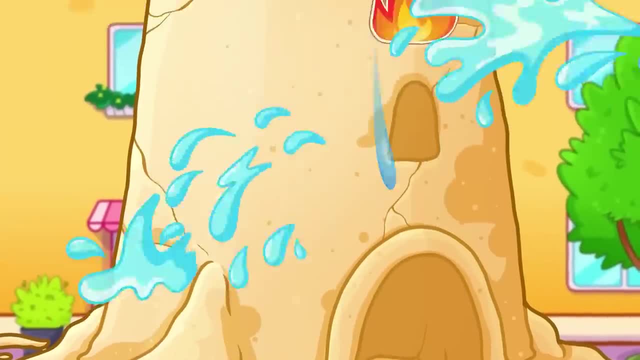 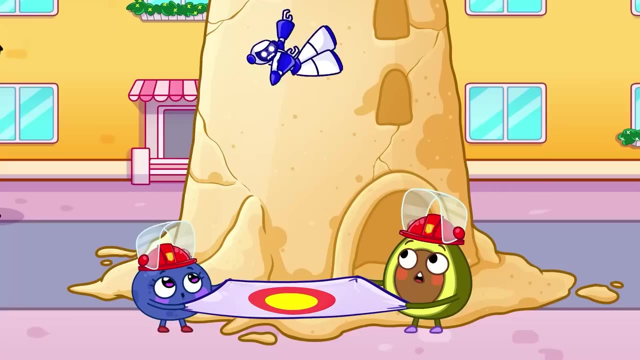 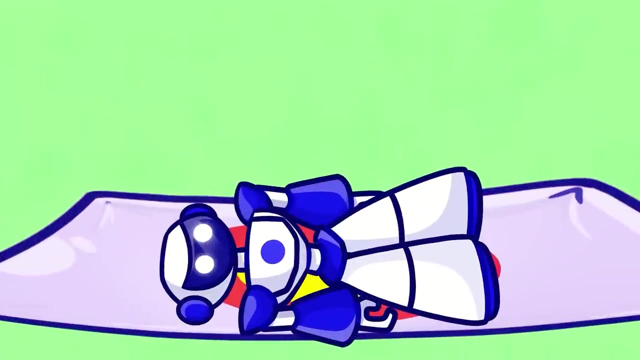 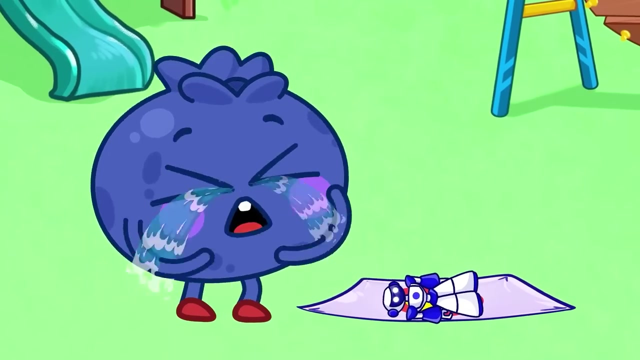 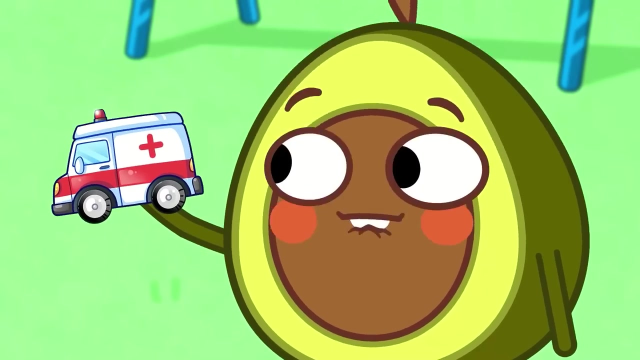 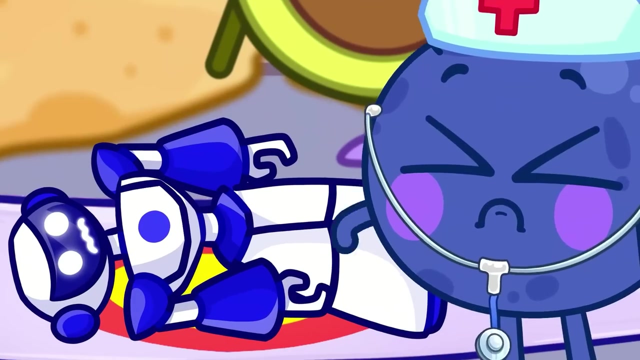 It's working. The robot is going to fall. Phew, You caught him, But now he doesn't work. Oh no, It's broken. Pit knows who can help. The nebulas will save him. Phew, His heart is not working. 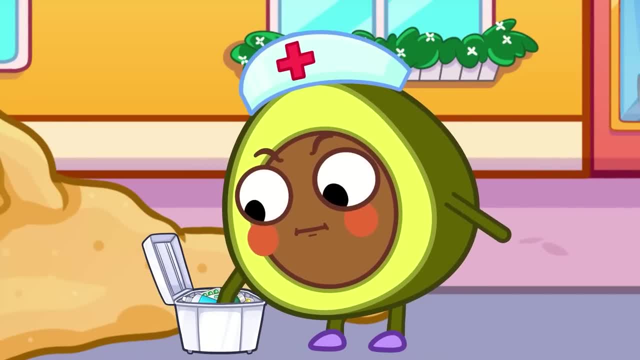 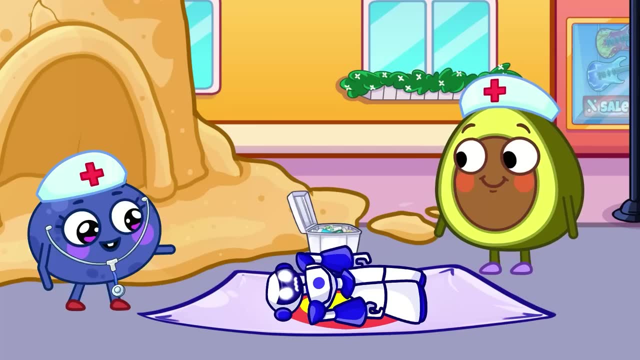 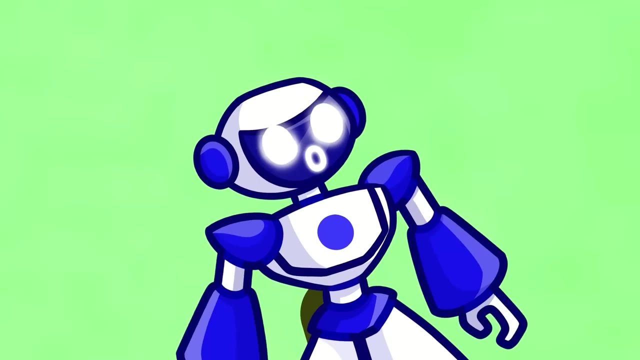 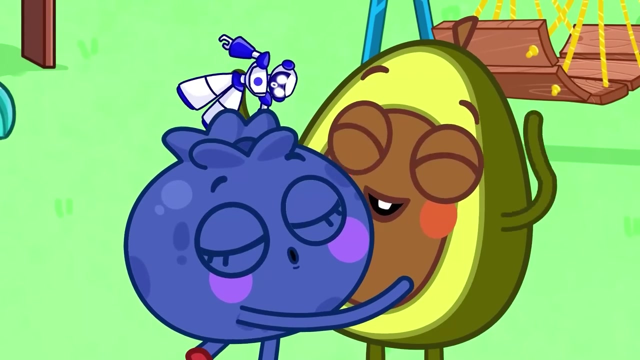 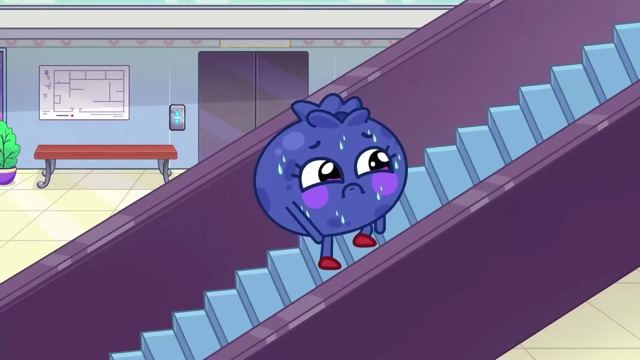 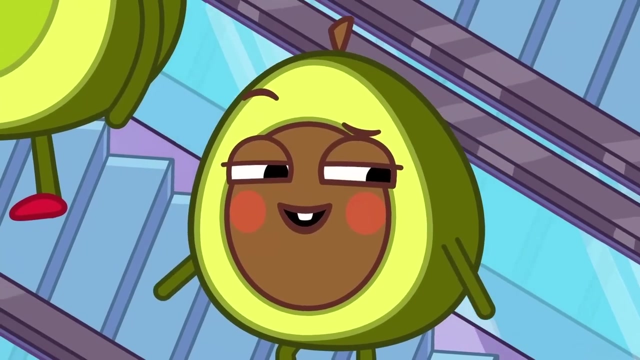 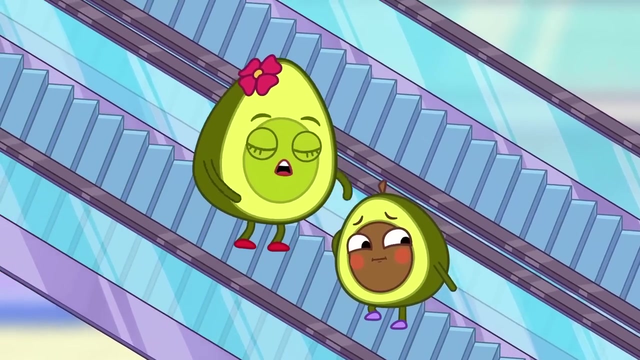 Maybe he needs some medicine. Yay, The robot needed new batteries. He's not broken, Blueberry, Thank you, Thank you, Thank you. Now he's ready for more adventures. she does this. you can't get distracted on the escalator. okay, I'll be. 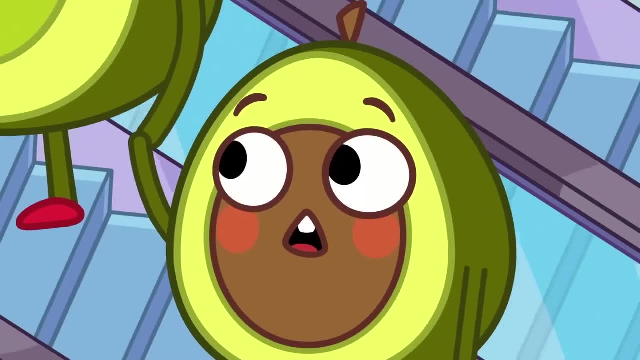 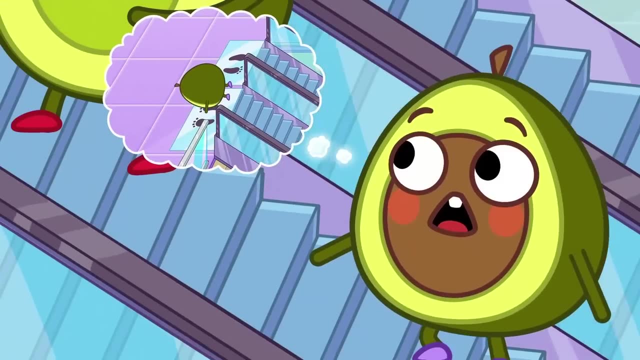 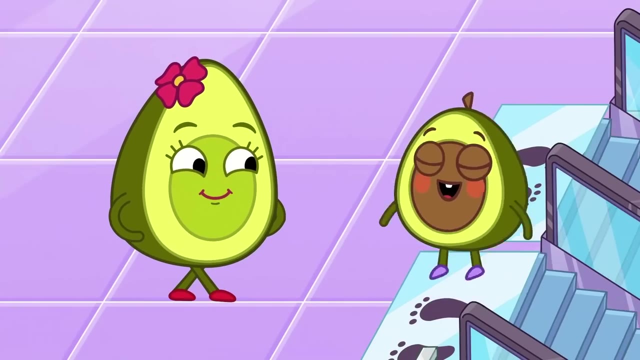 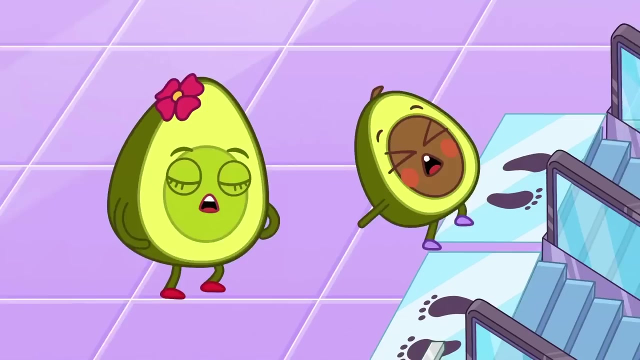 more careful. I'll stay nice and still, oh no, the top is so scary I might trip. what should I do? I'll be brave. I did it. I like it. I want to do it again. I'll just hop back. I need to use the down escalator. 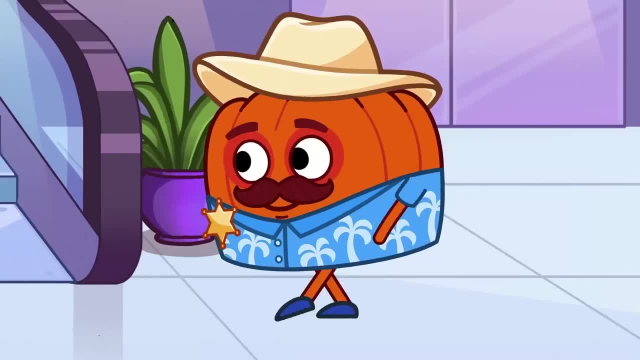 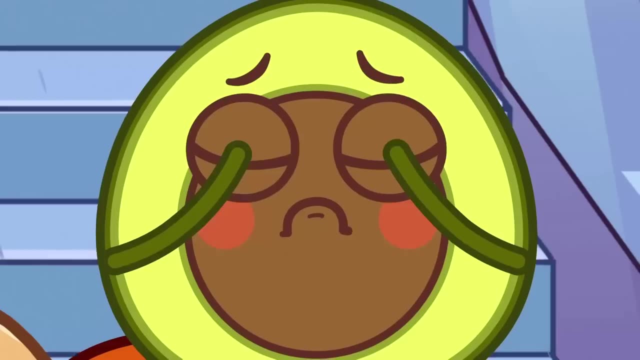 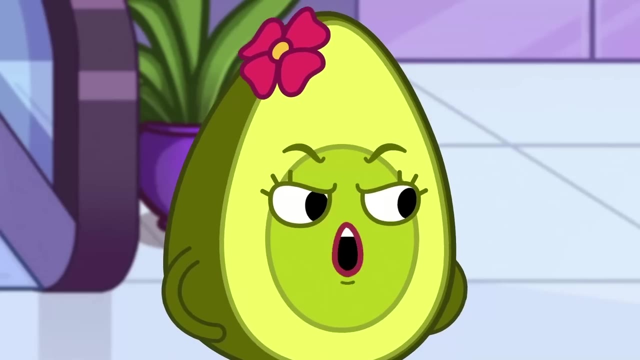 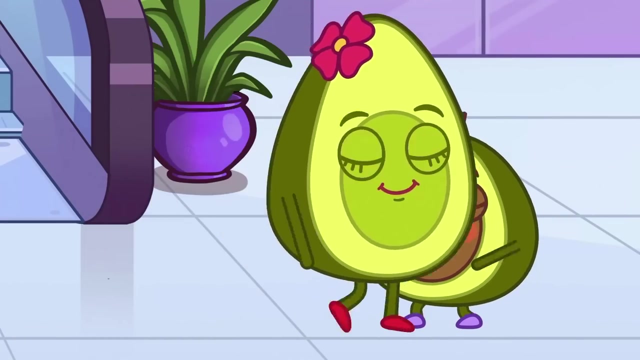 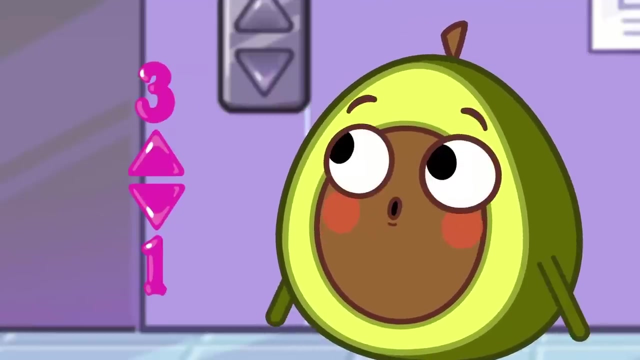 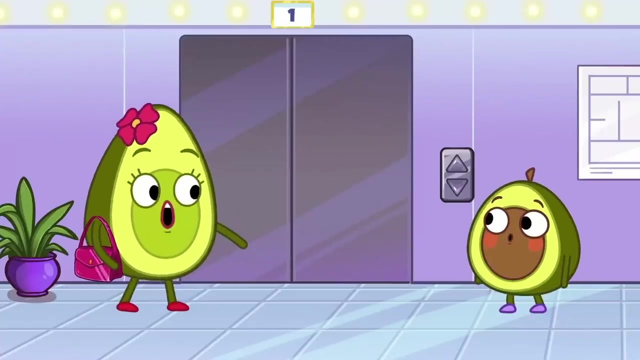 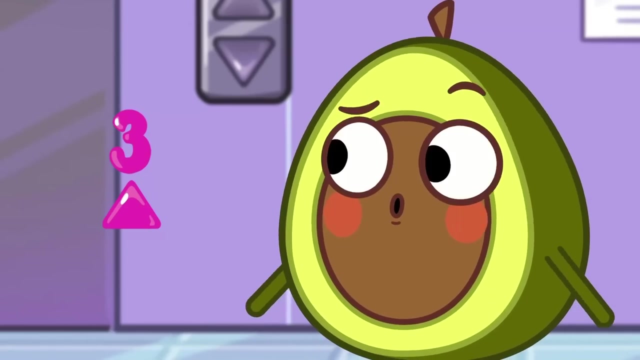 am I okay? don't run on the escalator. I'm sorry, I won't run on the escalator. we need the third floor. do I press B the up or down button? what does the one mean? that mean the elevator is on the first floor. so which? but you choose the direction. we need three is higher. we 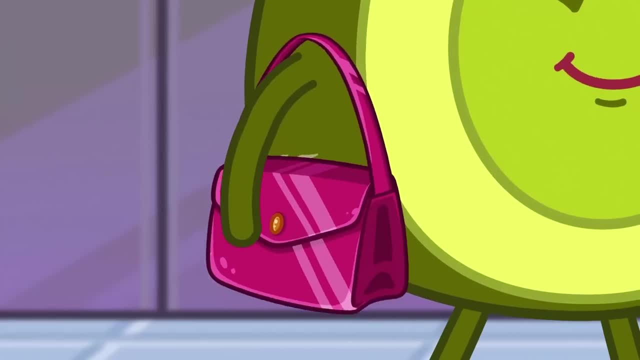 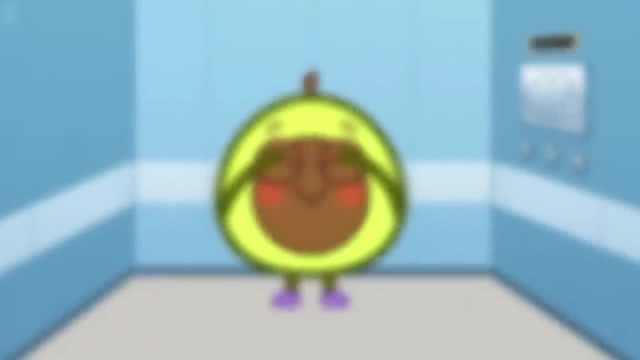 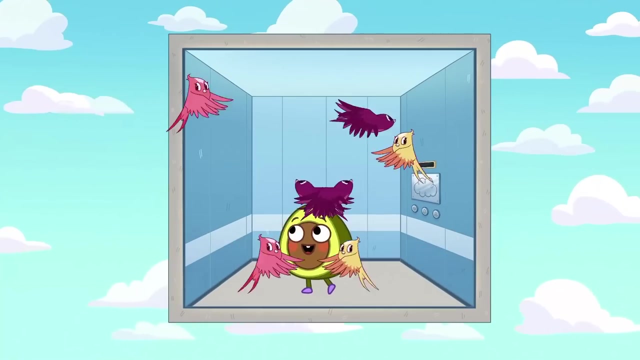 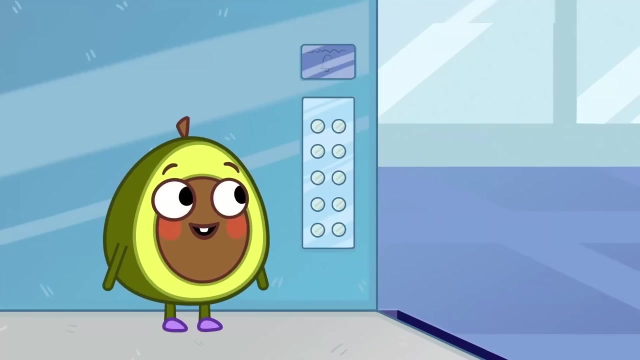 need the up arrow. Tommy, your purse broke. I know I'll take the elevator all the way up the escalator. I know I'll take the elevator all the way up the escalator to the clouds, hello birdies. to the clouds, hello birdies. now's my chance. which button should I press? I'll press the wall. 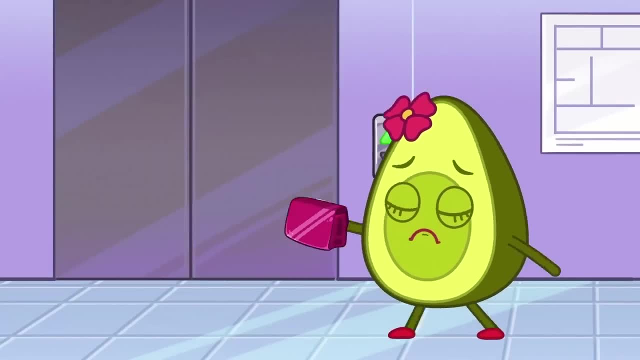 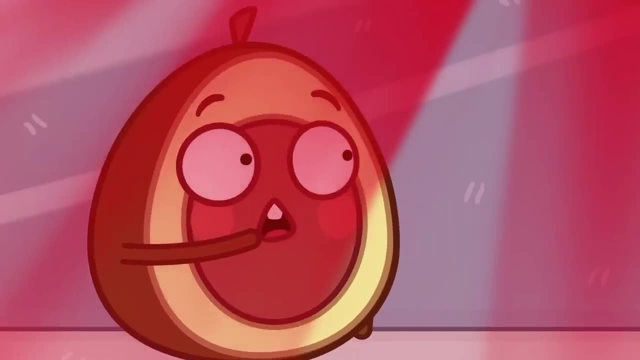 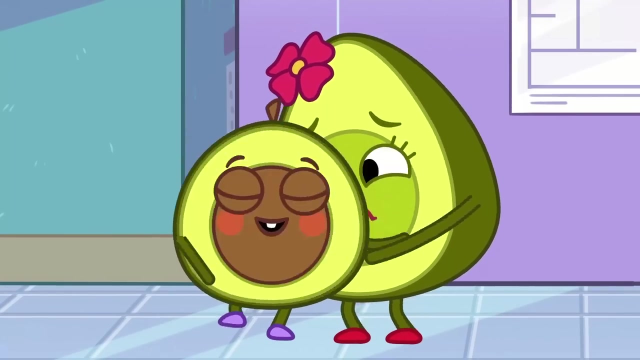 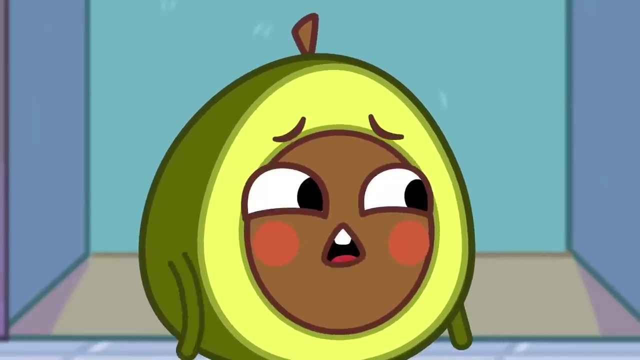 now's my chance. which button should I press? I'll press the wall. bye, mommy. oh no, what did I do? a monster's trying to get in, oh no, what did I do? a monster's trying to get in, mommy? oh, and, thank you, mr potato. oh, I'm sorry, mommy, I won't play in the elevator again. 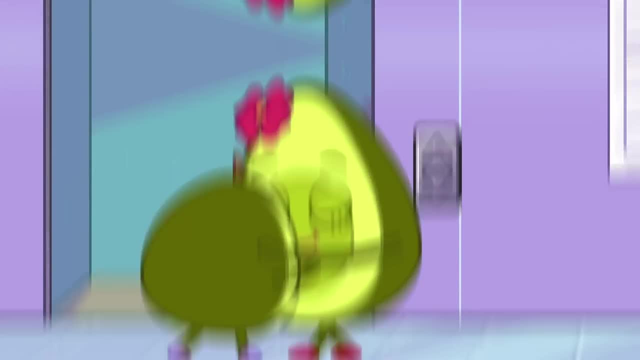 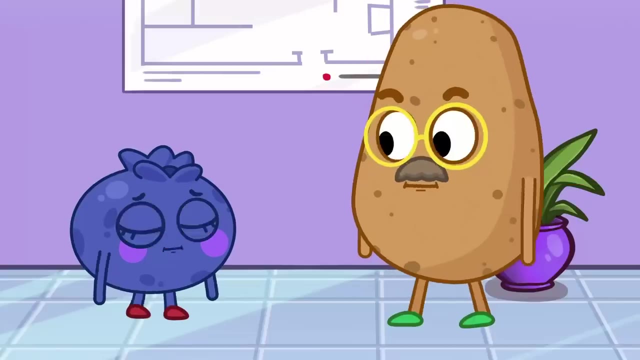 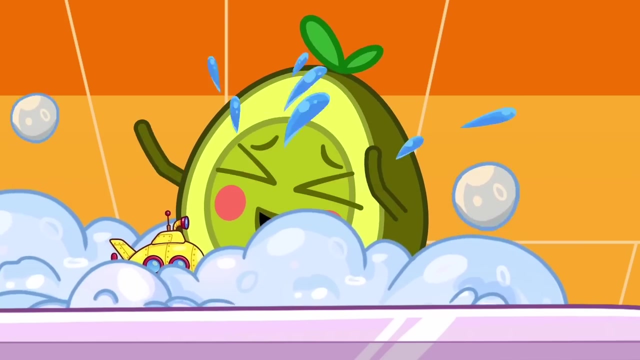 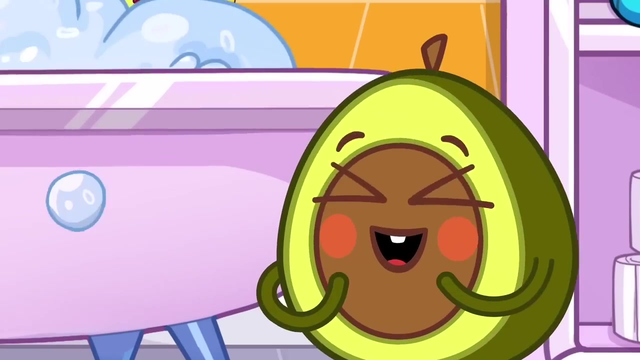 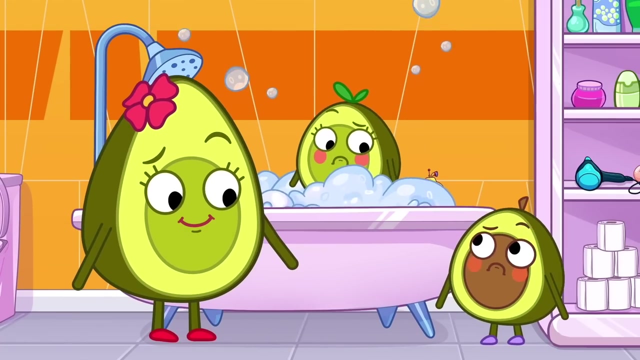 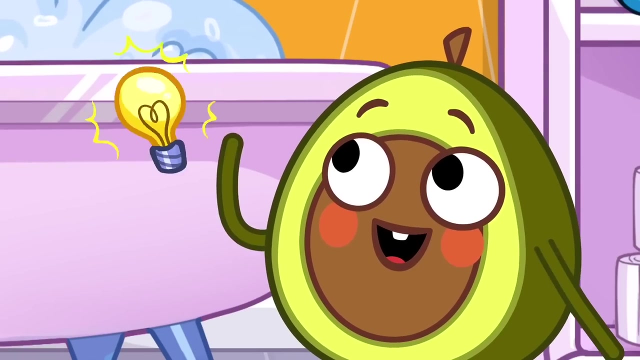 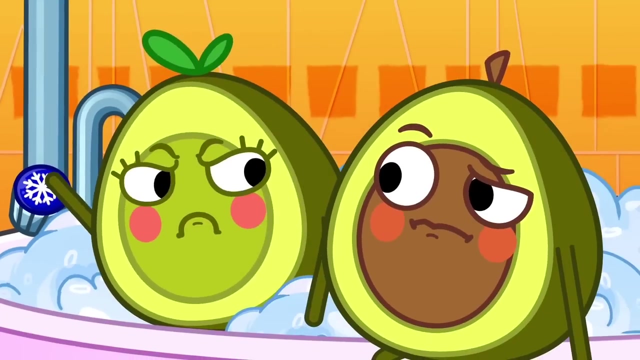 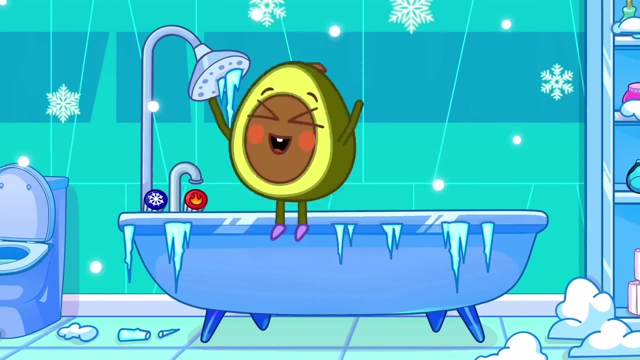 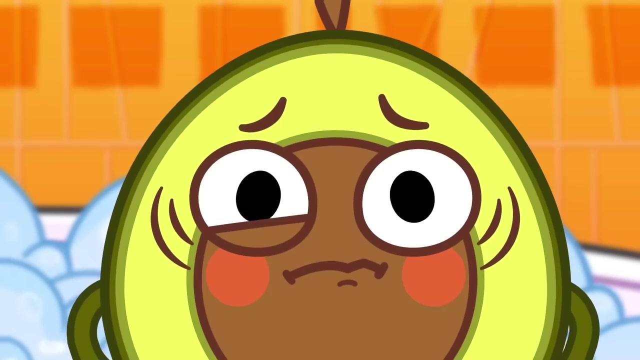 oh, oh oh. Penny is playing in the bath And here comes Pit Kids. Did you see a thermometer? What are you thinking, Pit Pit, don't play with the faucet. That one will make the water too cold. Penny, don't play with the faucet. 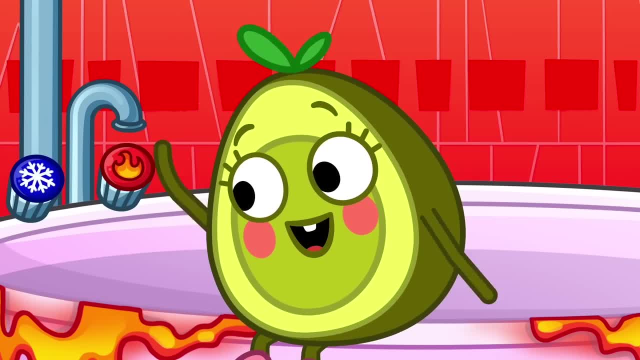 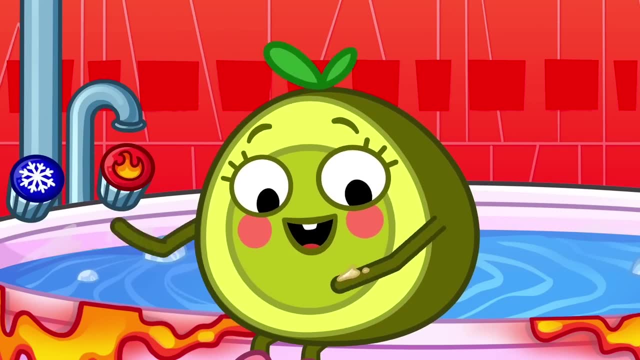 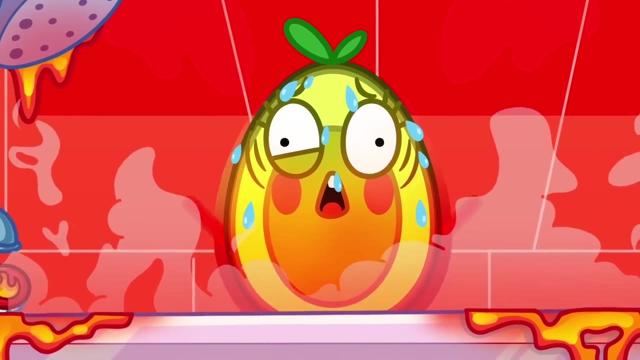 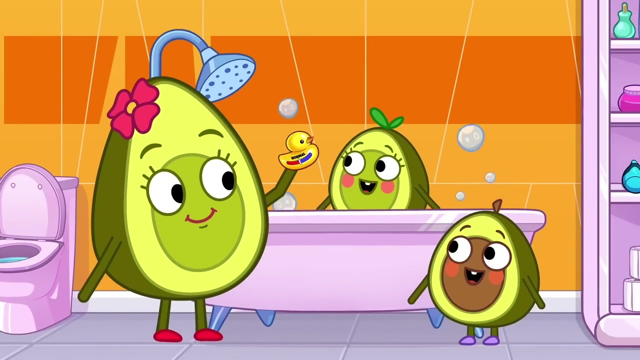 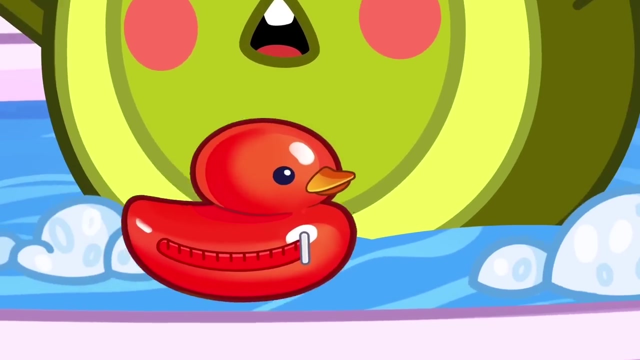 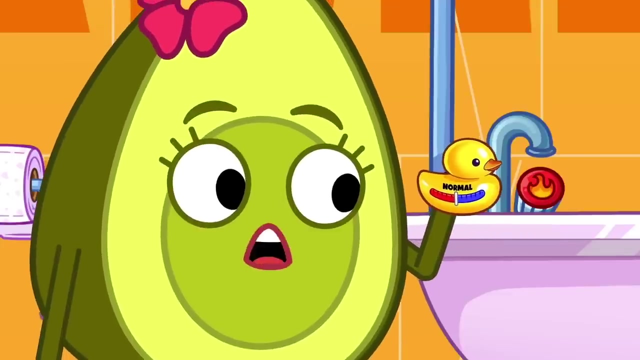 And that one will make the water too hot. Here comes Mommy. She will see if the water is too hot or too cold. The bath is too hot, So Mommy adds cold water. You can take a bath. You can take a bath. 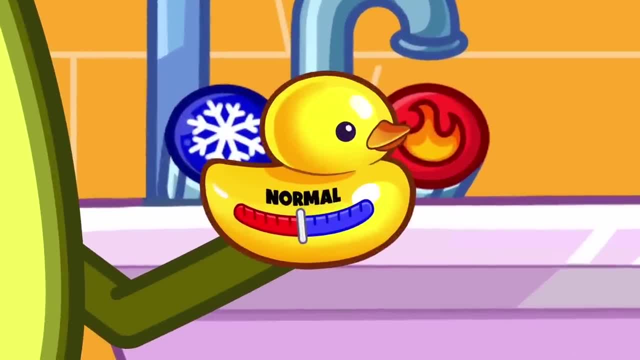 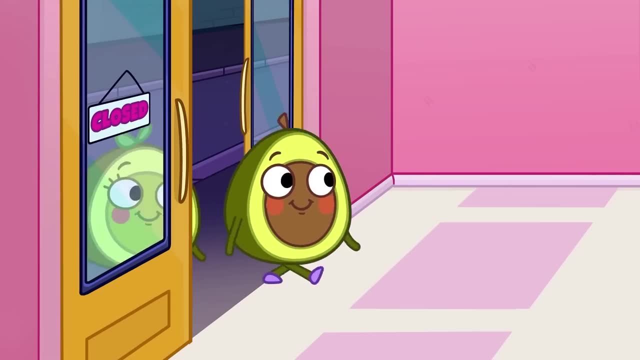 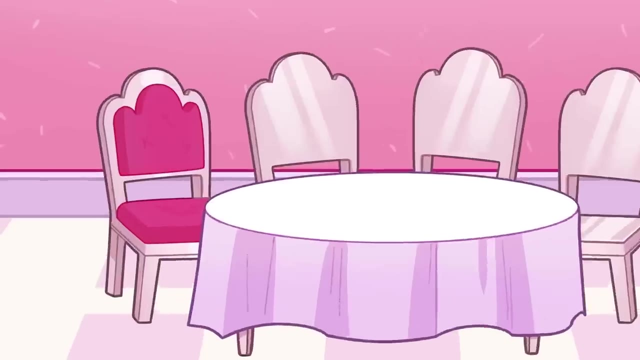 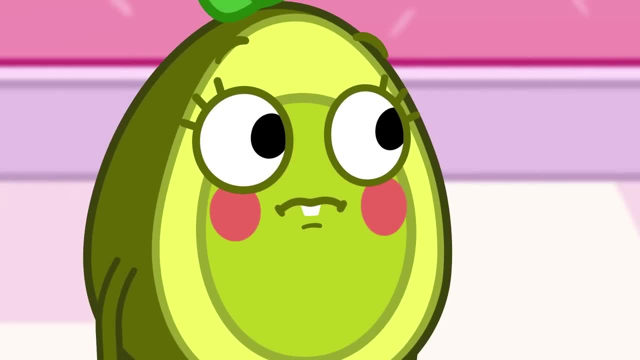 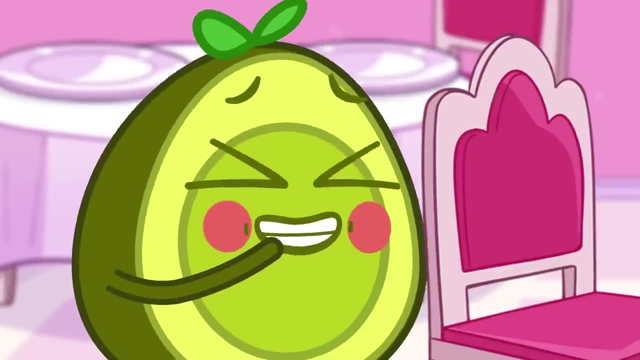 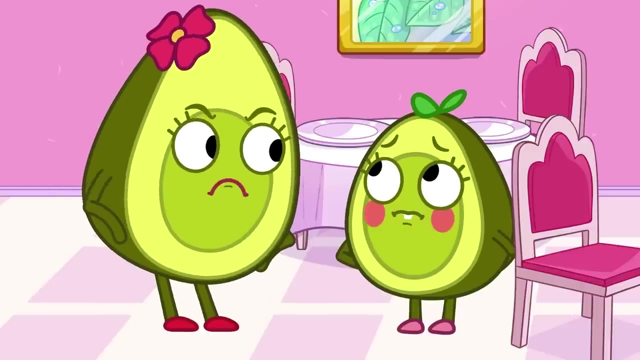 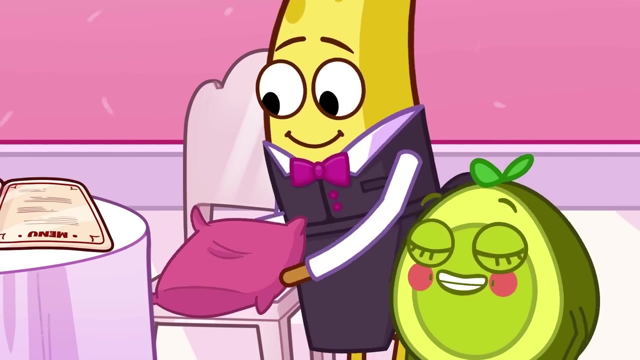 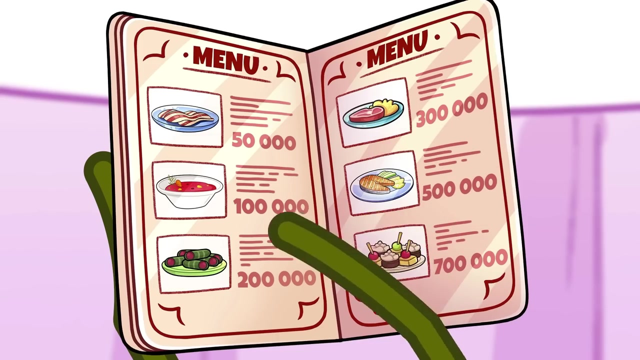 And Pit got it first. No, Penny, Not that one. Mr Carrot was using it. Kids, if you have a problem, call the waiter. You can sit here, Penny. What's on the menu? Pit? Pit wants to try being a chef. 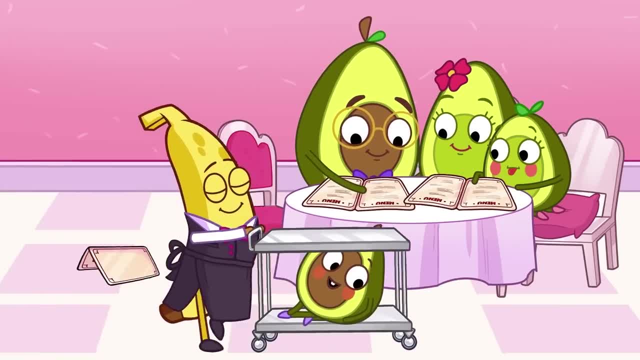 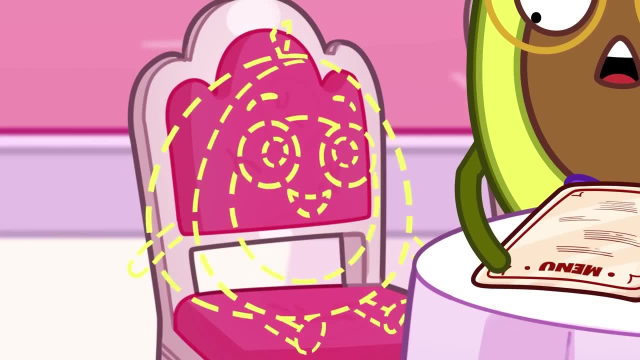 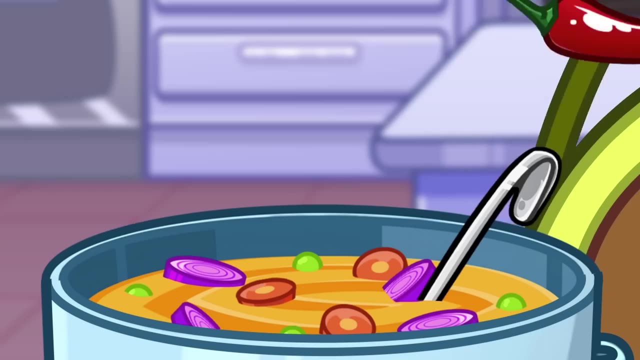 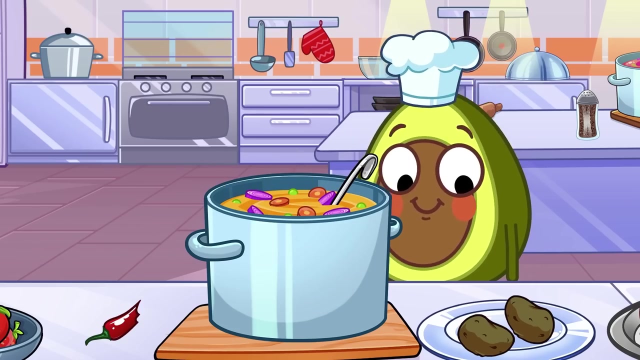 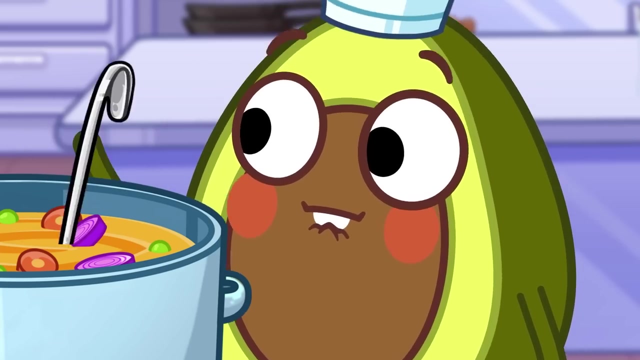 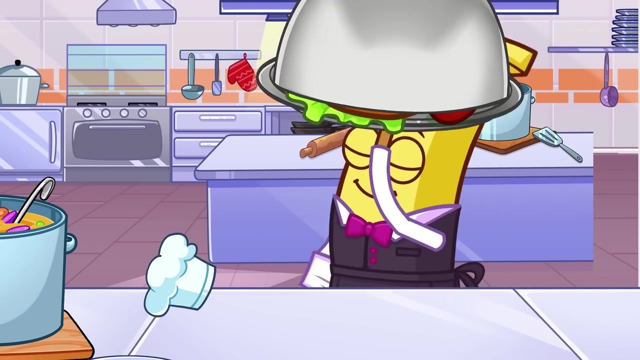 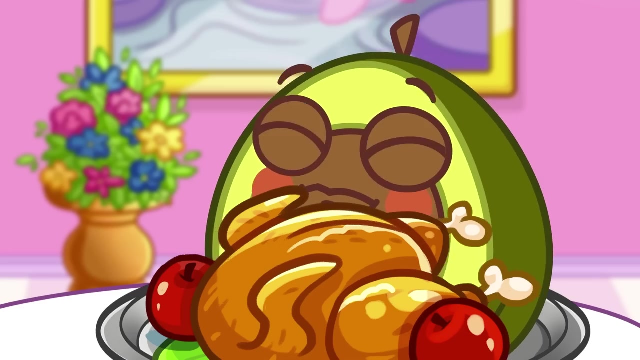 Now, what is he up to? Pit, have you picked what? Pit's not there, Daddy? He's in the kitchen to be a chef. Pit, that's not your soup, That's it. Here comes the waiter. Oh, Hurry, Daddy Pit's over here. 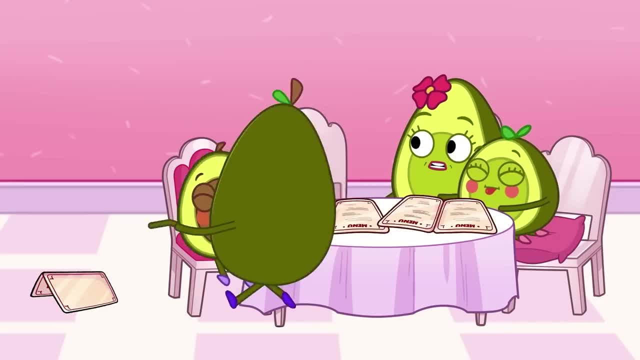 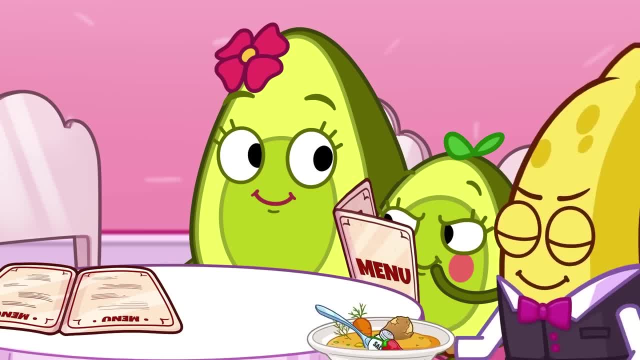 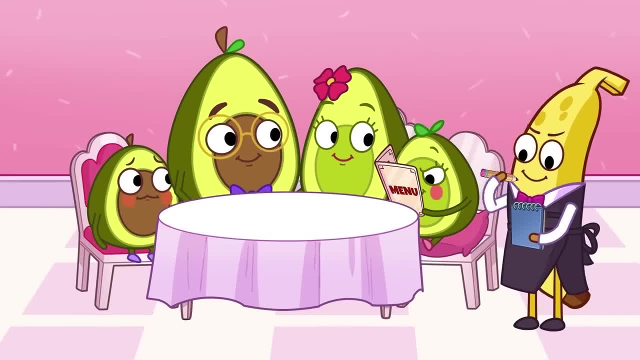 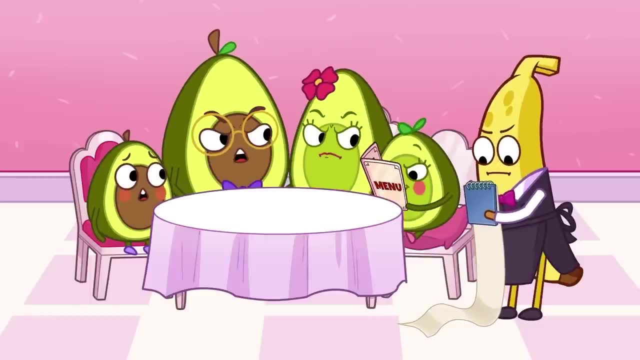 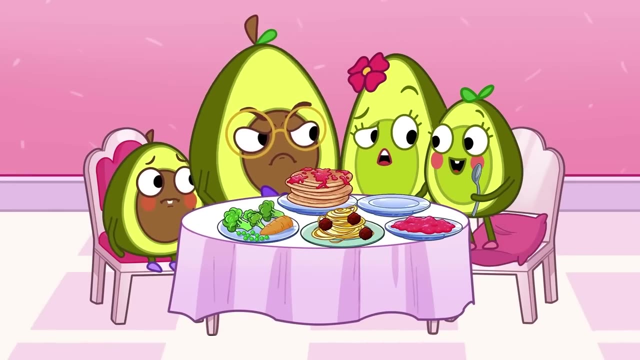 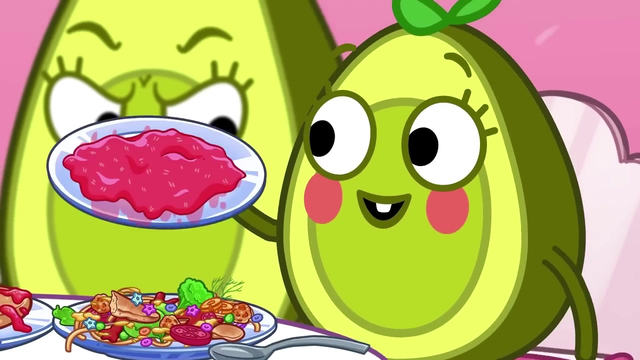 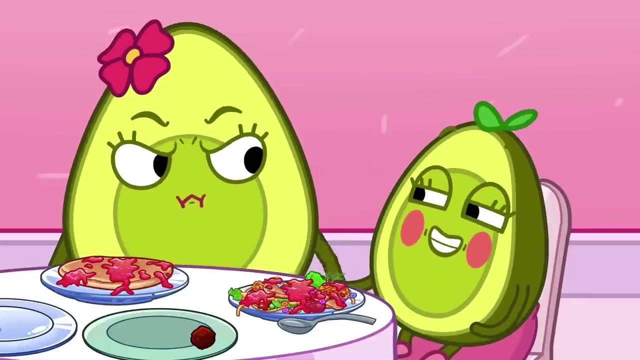 What would you like to order? Penny? Everything, Penny. it's too much for you. Only order what you can eat. Oh, no, Oh, Oh, Oh, Oh, Oh. Penny, mixed together all the food. It looks terrible. Don't mix the dishes. eat them one by one. 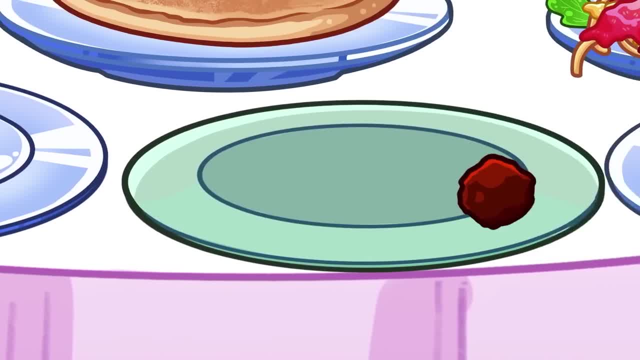 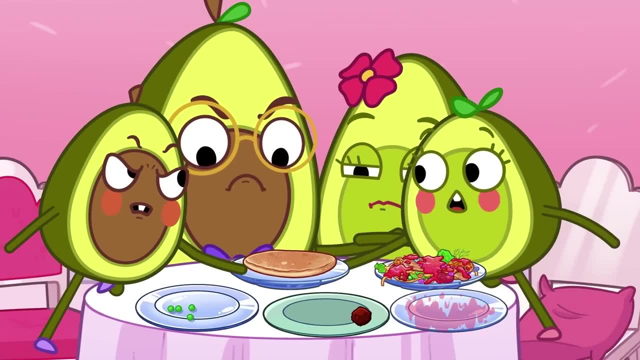 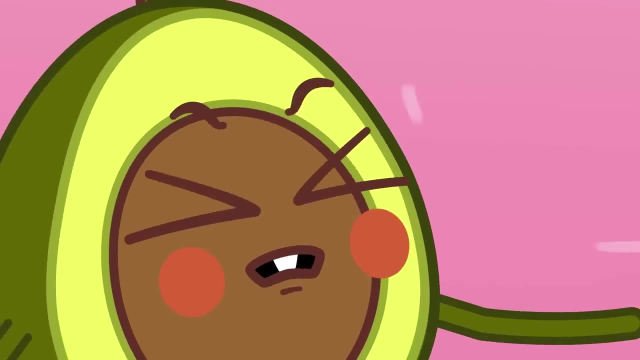 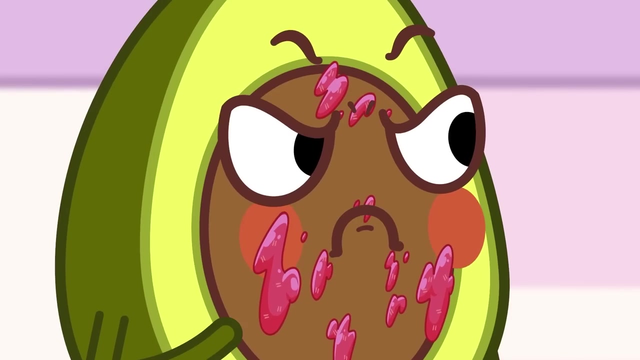 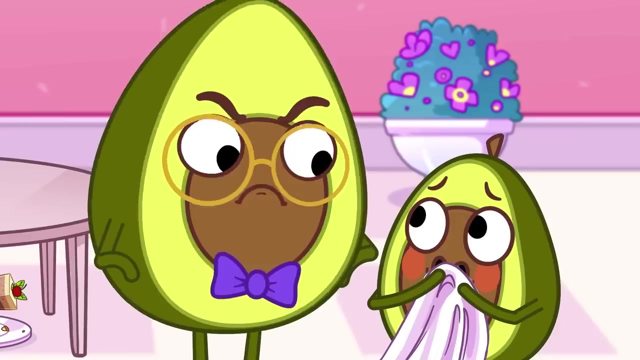 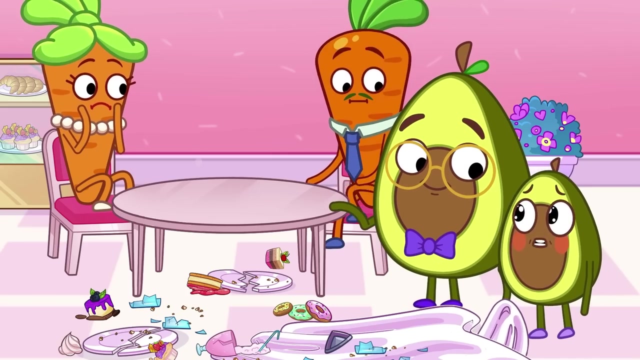 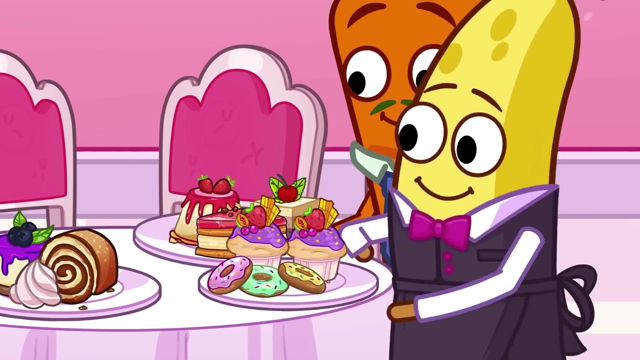 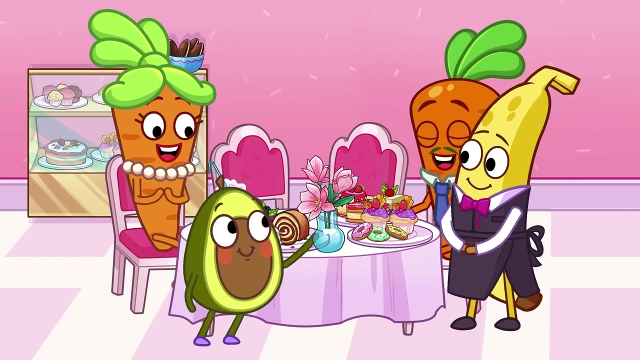 There's one pancake left, But both kids want it. Oh no, Now look at this mess. You can't damage the restaurant and disturb other visitors. I'm so sorry. Pit wants to fix it. Pit makes his mistake. One final touch That's much better. Here comes lime. 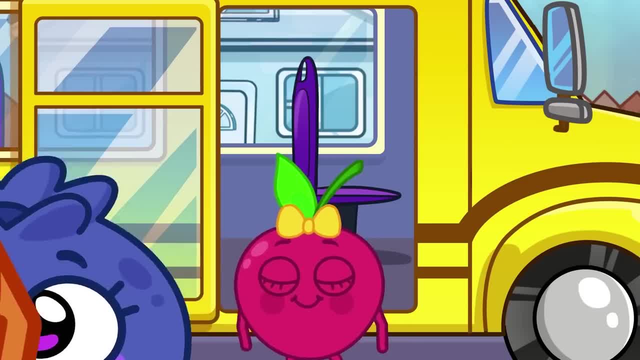 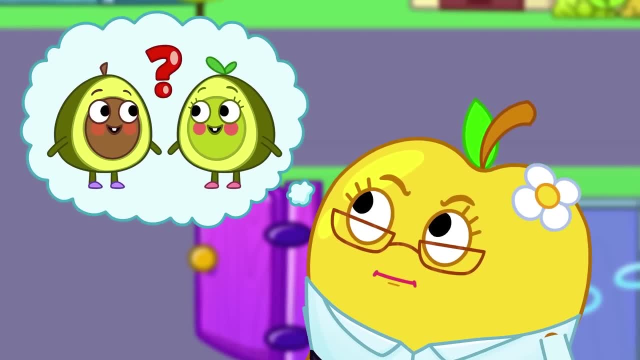 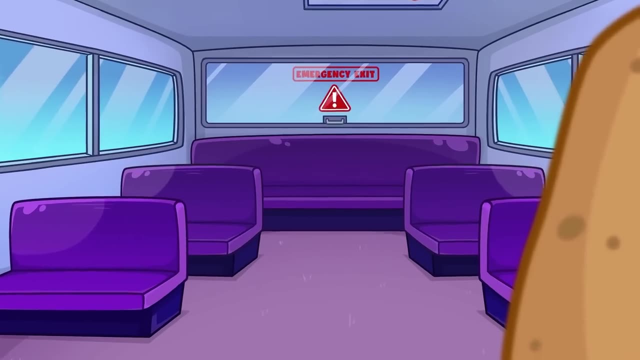 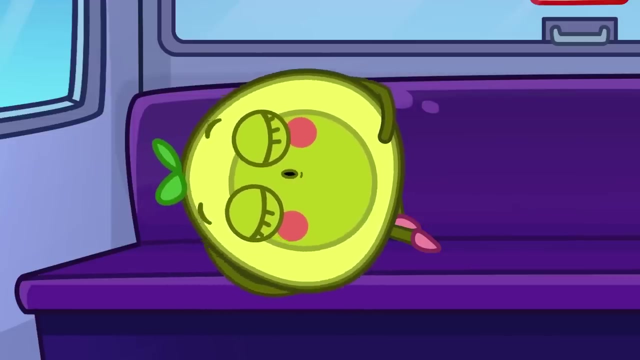 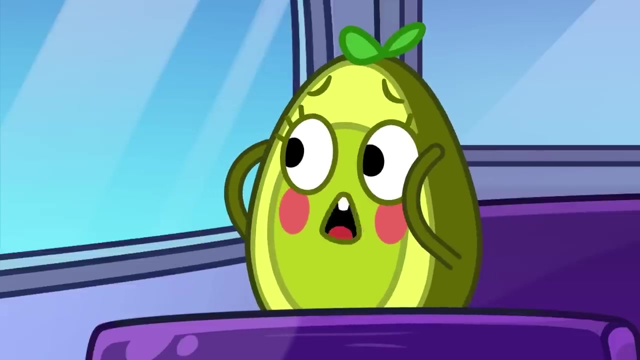 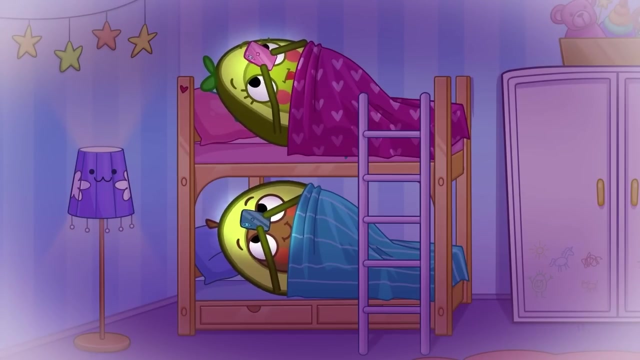 Perry, blueberry and cherry. Wait, Pit and Penny are missing. Otto doesn't think anyone is on the bus. Wake up Penny. We have slept throughout the stop. Pit and Penny stayed up late playing video games. Then they were right, They were really tired in the morning. 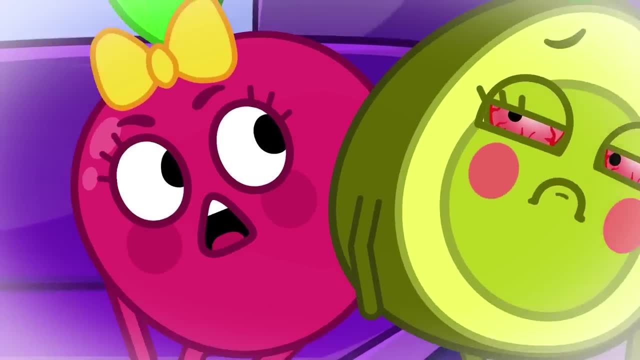 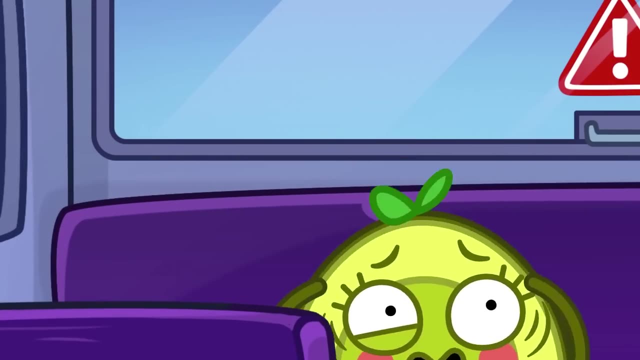 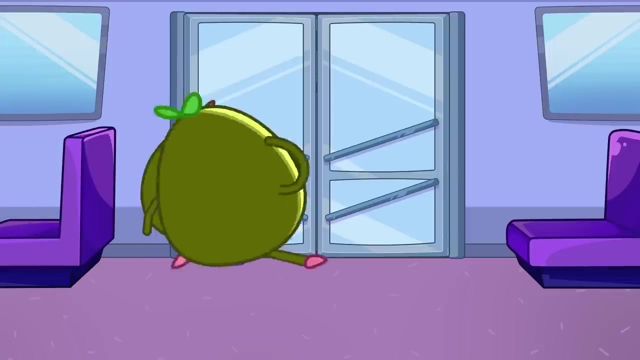 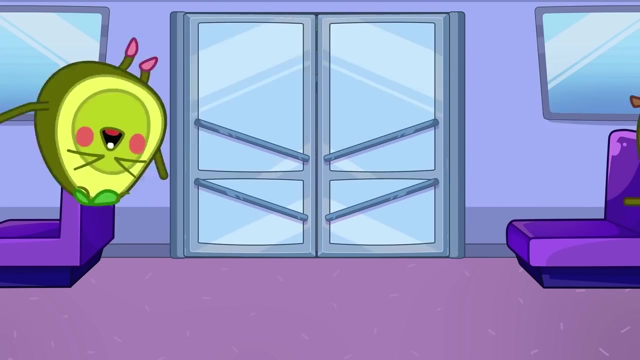 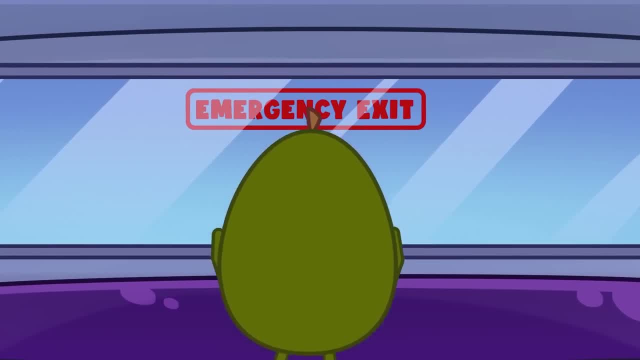 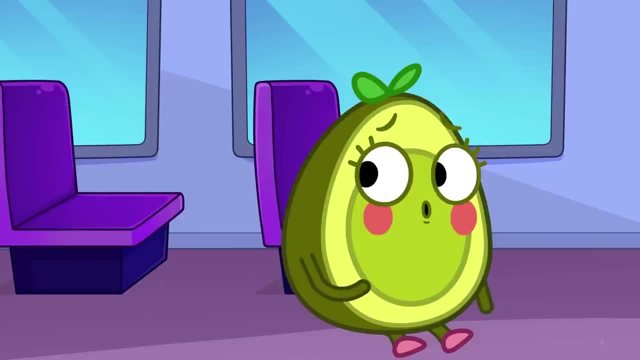 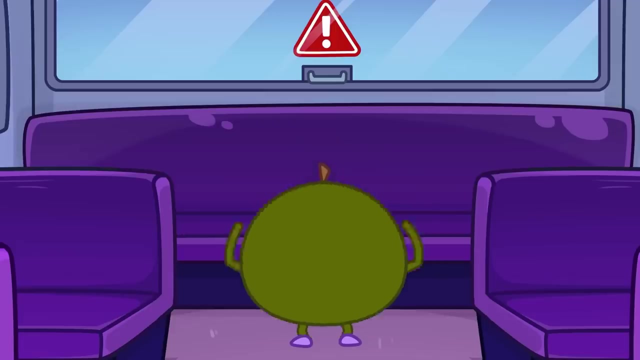 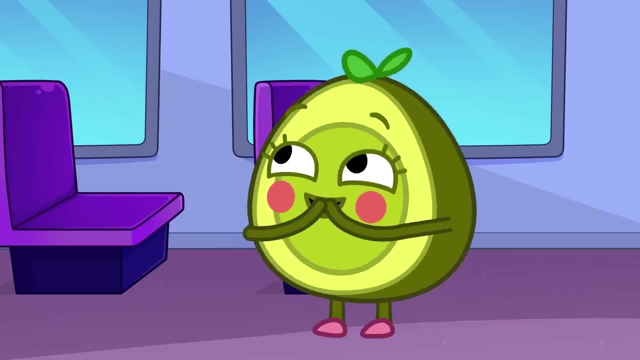 Oh no, Oh no, Oh no, Run Run. Fortunately they stayed at the footbridge. No, We are locked. Is there another way to get out? Hmm, Yes, there is an emergency exit. Oh, my, My needs, That's it. 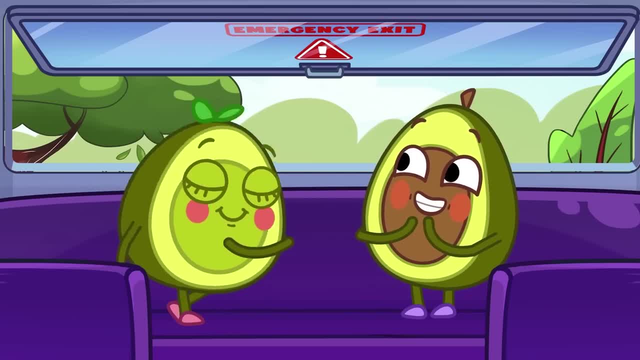 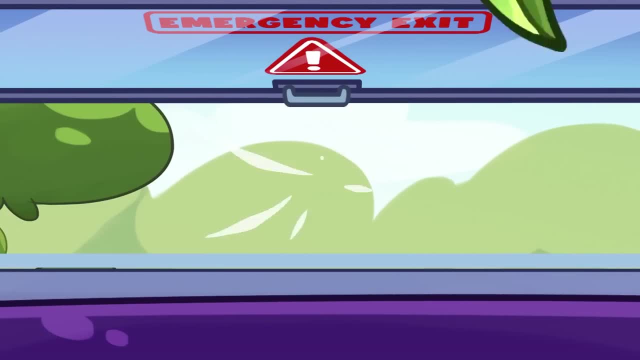 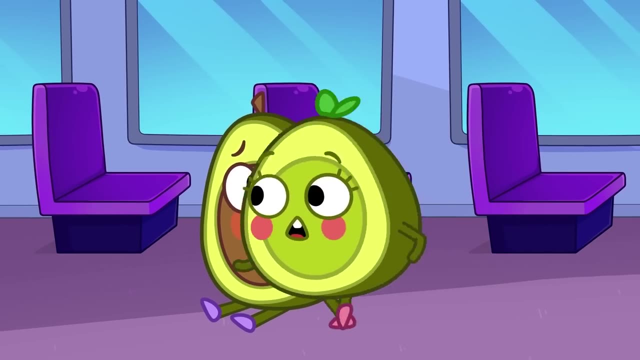 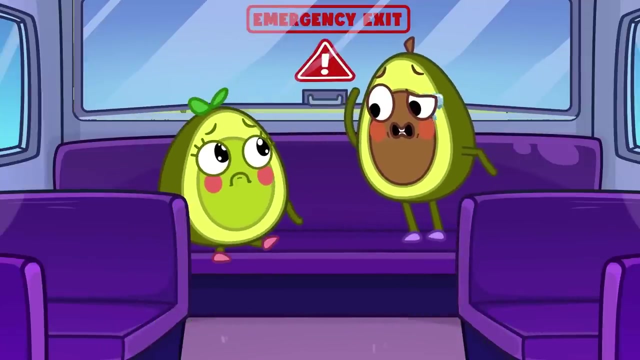 We are done. See you when the bus comes. Bye, Good night, Good night. Goodbye, Good night, No, no, Well done, Penny Hooray. We are free. The wind is too strong and it blocked the exit. Now it's stuck. Maybe there's another way out. 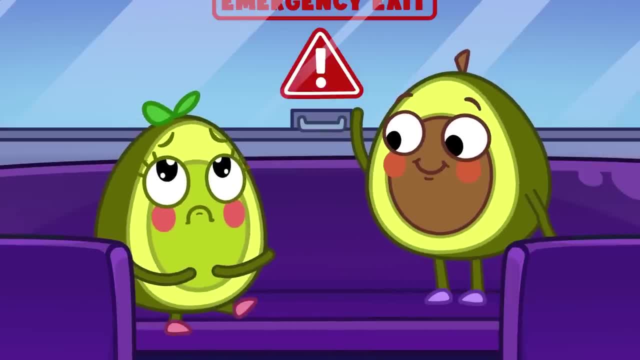 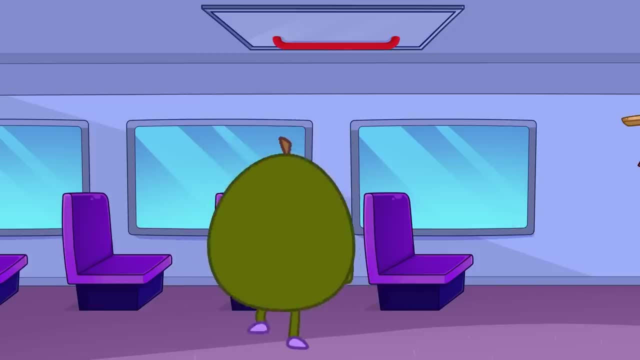 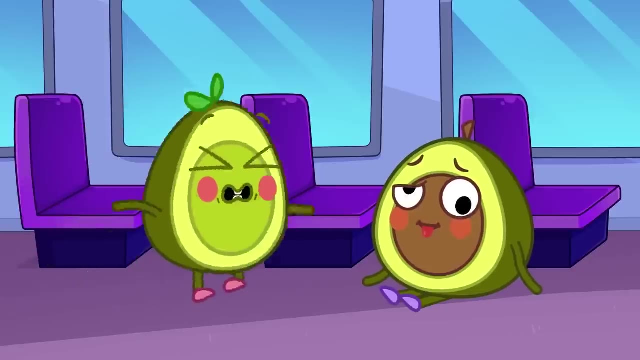 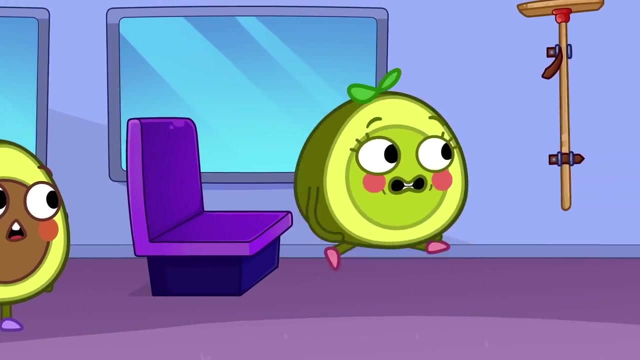 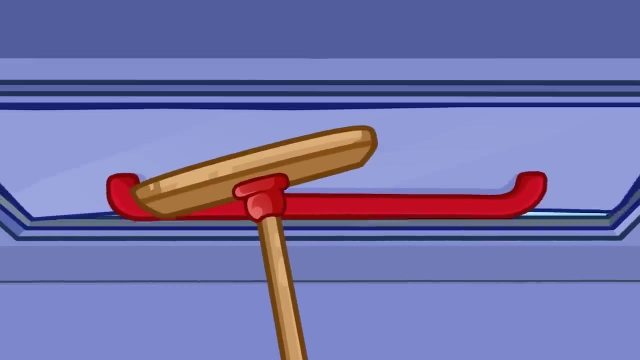 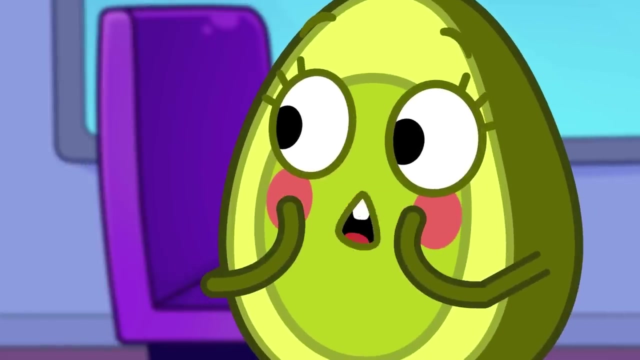 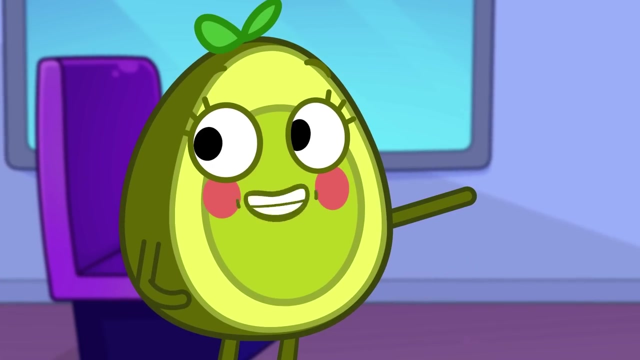 There's also a hatch in the roof, But how will Pit reach it? Be careful, Pit. Can you think of something? Penny The broom can reach the hatch, But how do we get to this hatch? Great, So adults can hear us. 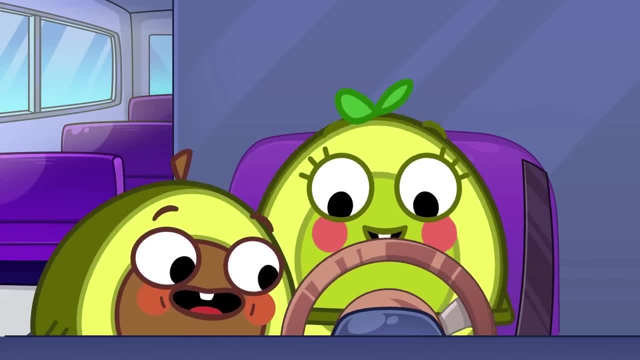 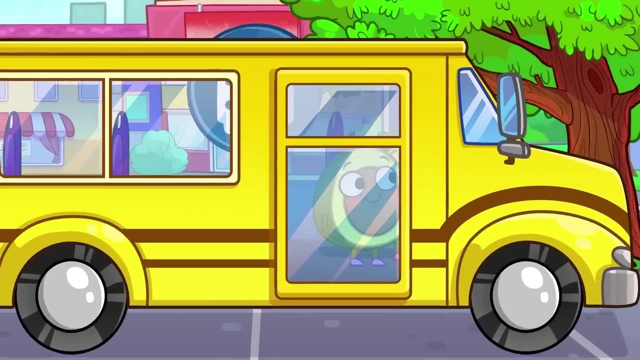 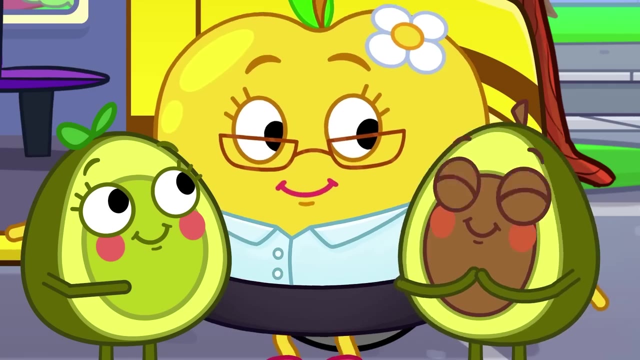 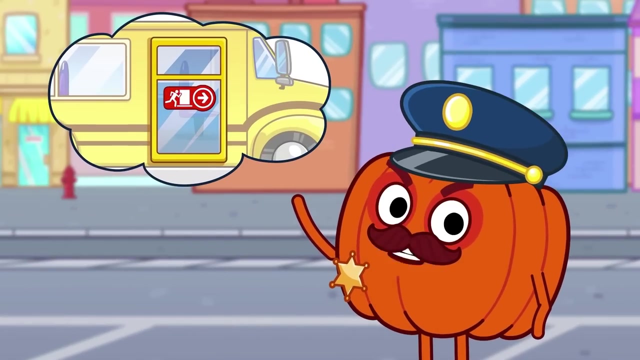 Honking the horn is a great idea. Officer Pumpkin and Miss Apple can hear the honking. Pit and Penny are safe. You saved us. No, you saved yourselves. If you're stuck on the bus, use the emergency exit immediately, Or use a horn to send a signal to an adult. 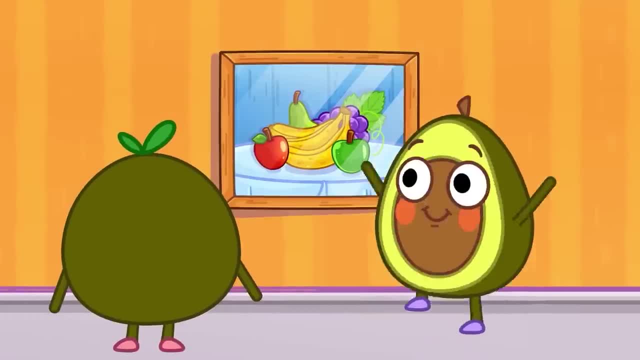 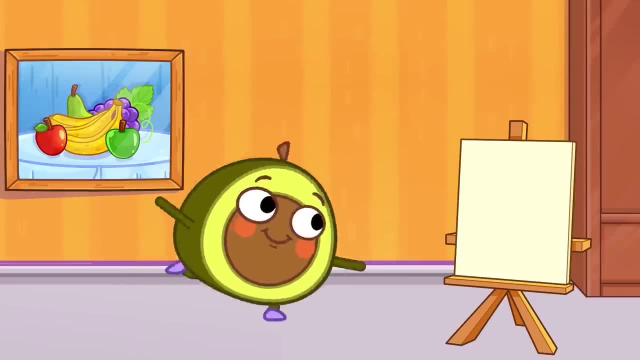 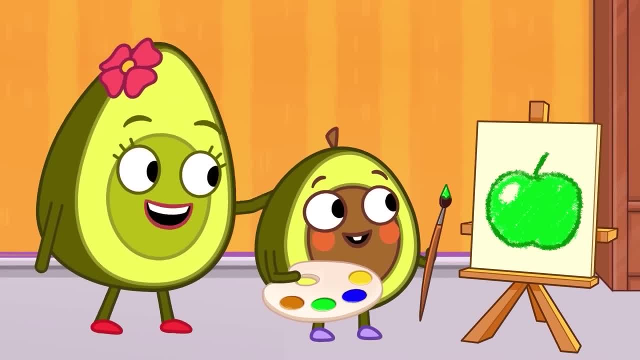 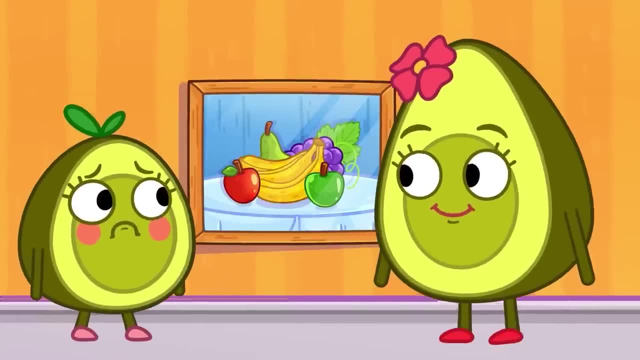 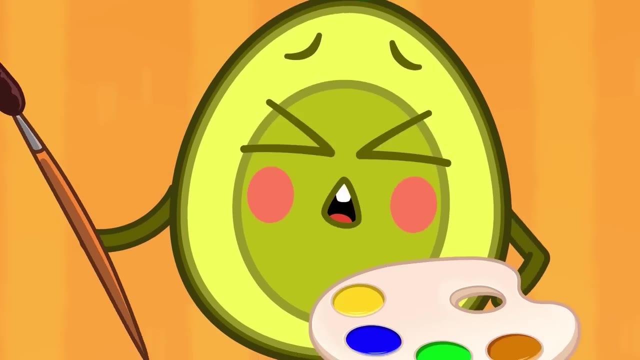 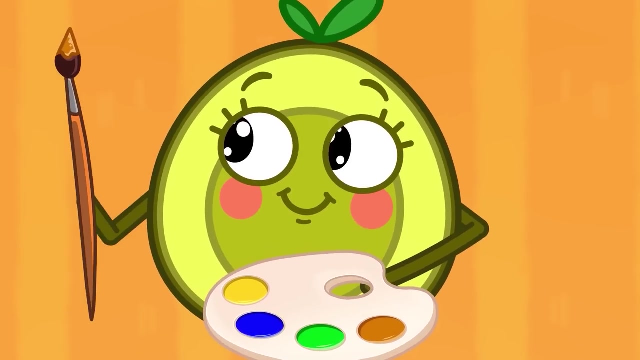 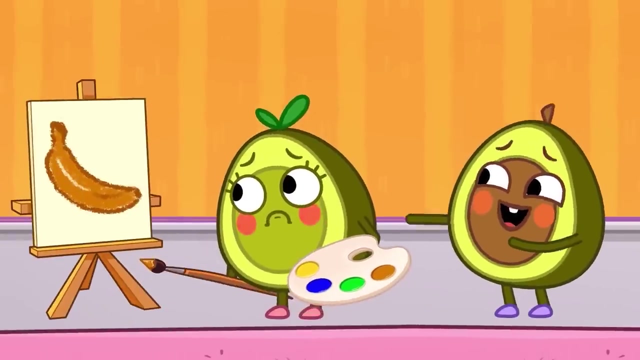 Pit starts to paint an apple. Well done, Pit. What's wrong? Penny, It's yellow. Penny. Now it's Penny's turn to paint. But what color is yellow? Yellow Penny is painting a banana. Penny, it's brown. 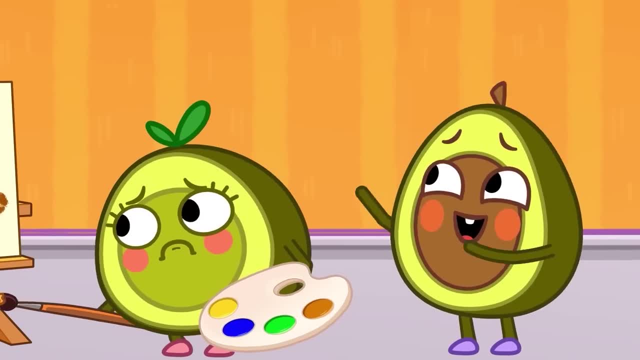 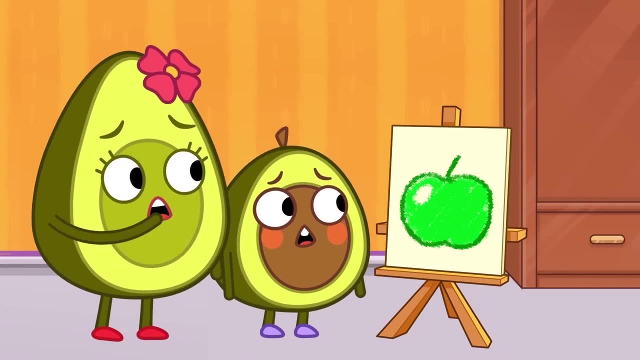 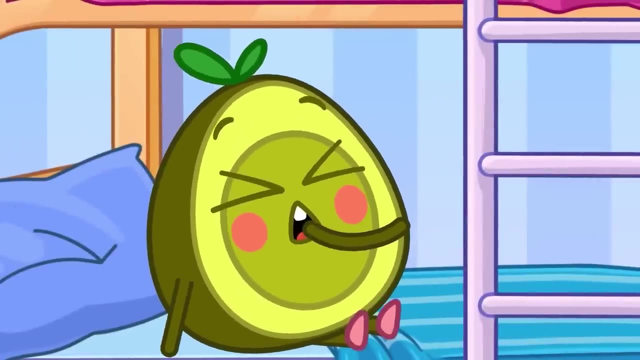 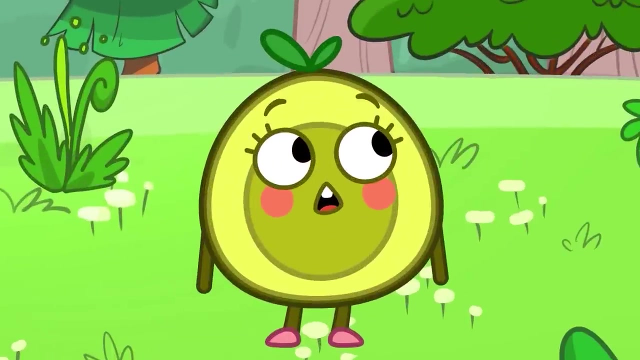 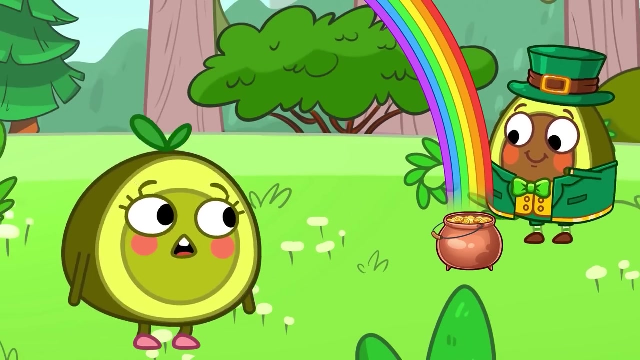 You need yellow paint. Oh no, Penny is upset. No, I don't want to paint, I want to learn colors. It's boring. Penny is sleepy and starts to dream. Penny, What a pretty rainbow. But the rain clouds make the rainbow go away. 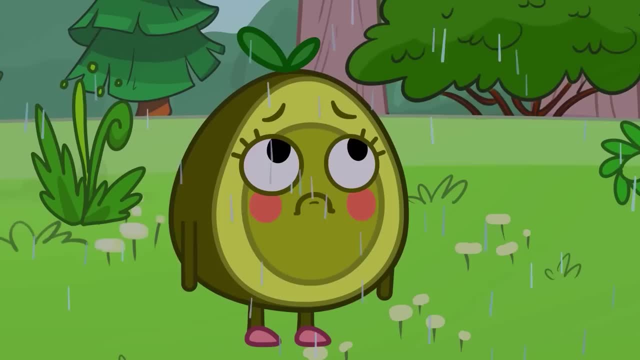 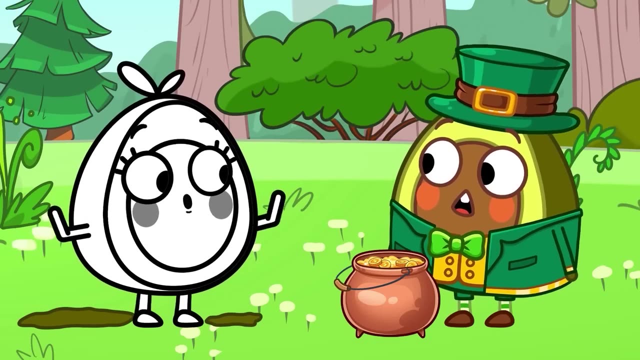 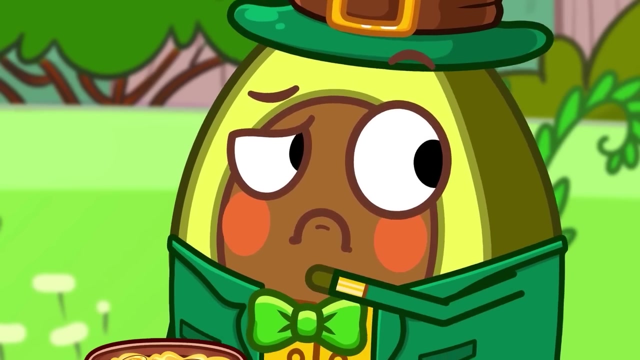 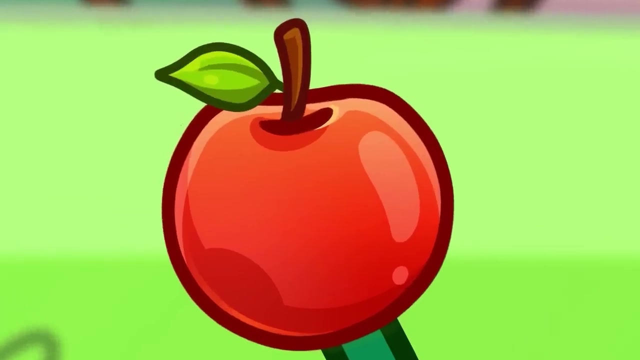 Oh, Pit and Penny are getting wet. Penny's colors are washing off. Ooh, I love my color. Wow, I love my color. Ooh, I love my color. Hmm, I have an idea. Pit has a crunchy red apple. 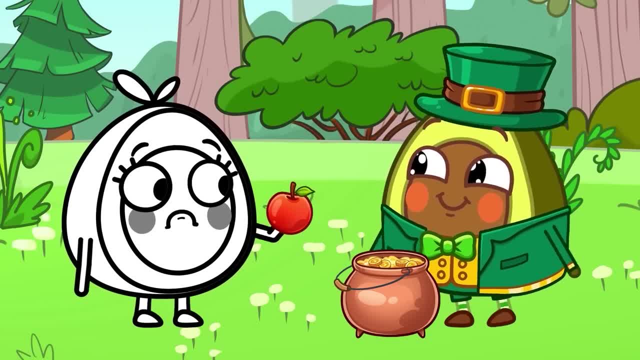 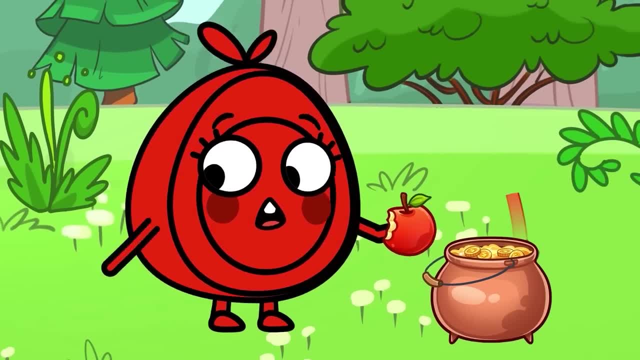 Pit has a crunchy red apple. Huh Yeah, Try it. Ow, Penny eats the apple. What, How? Penny eats the apple. Ahhh, It's so pretty, Despite the rain. It's not my color Because it's red. 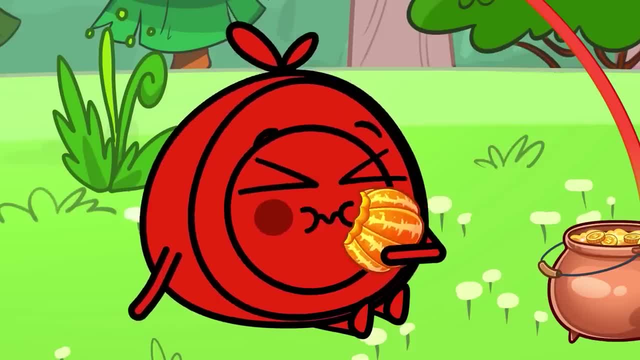 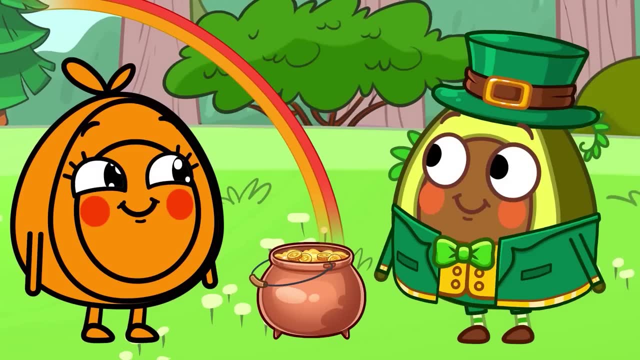 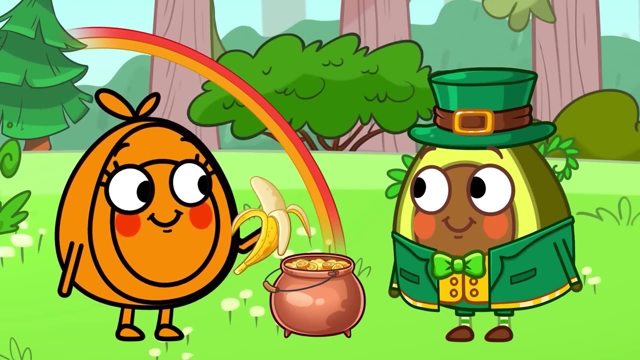 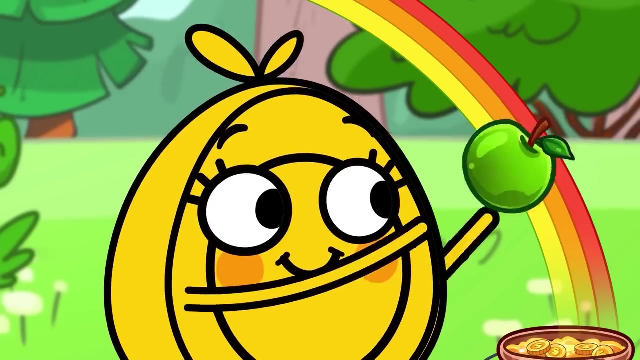 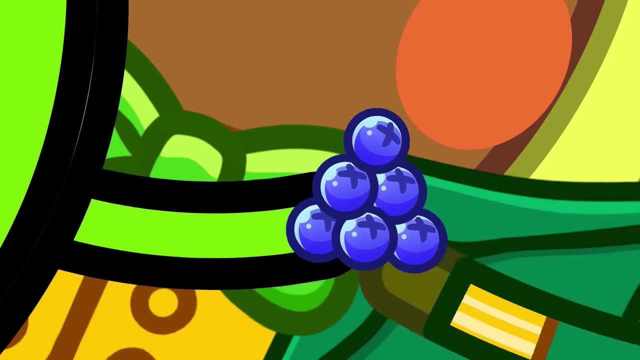 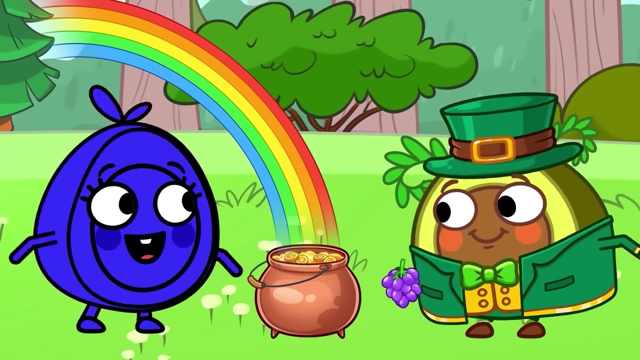 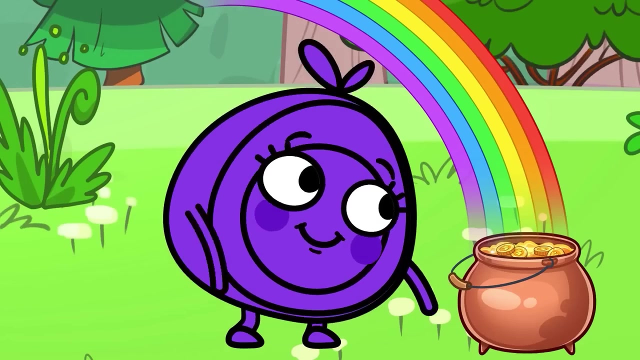 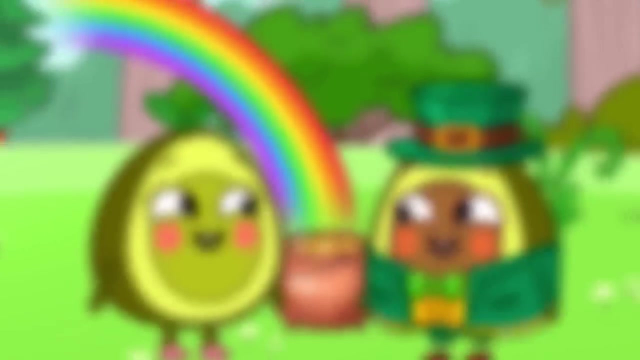 Hit with Penny and Orange. Penny has changed color. Wow, Hello, Penny is changing colors, just like the rainbow: Purple. Look, Penny, The rainbow has its colors again. I'm green, Woohoo, Yay, Penny, Penny. 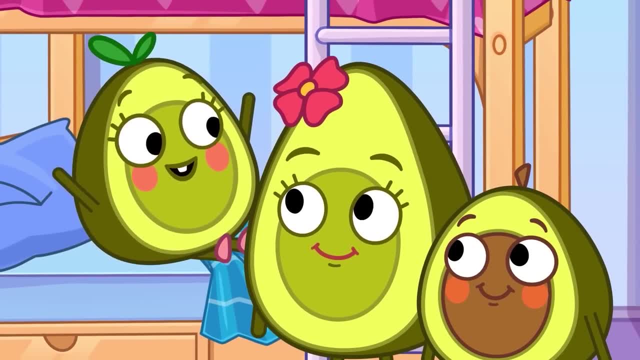 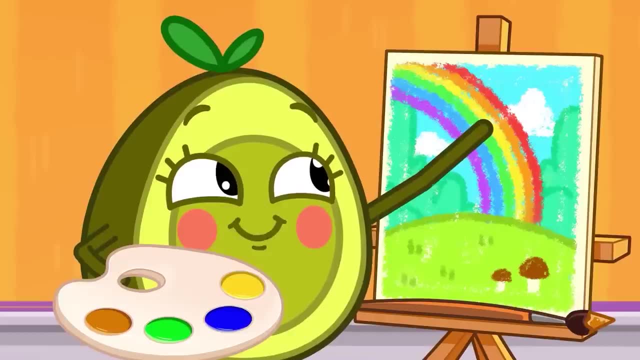 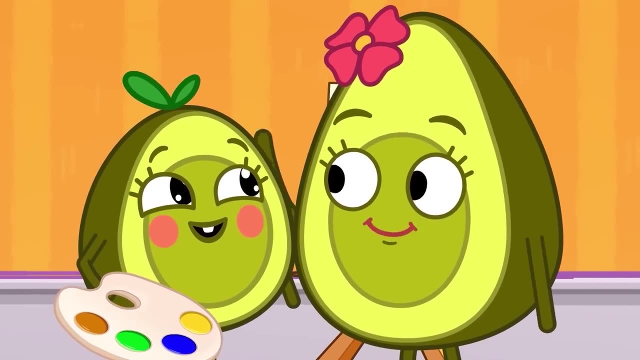 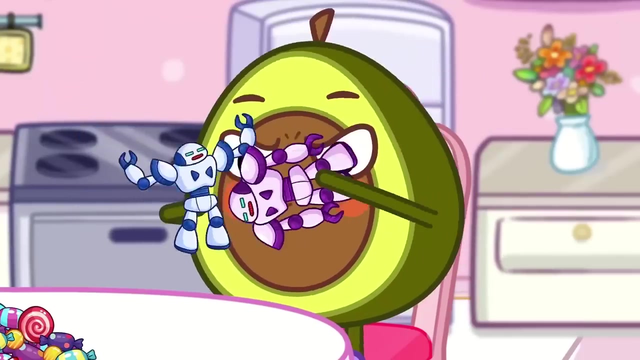 Huh, I want to draw. Oh, Red, Orange, Yellow, Green, Blue, Purple. Yay, Yes, that's right, I love Penny. Ah, Hit and Penny are playing with their toys. Penny loves dolls, Pit loves robots. 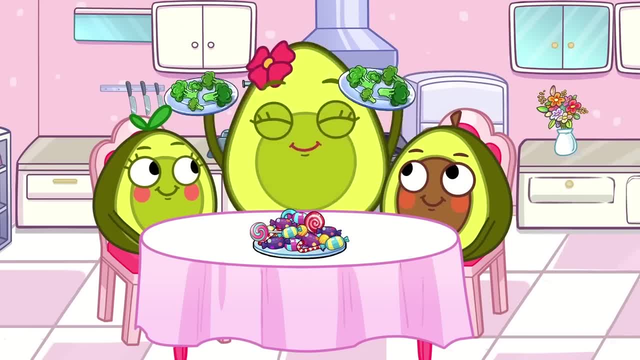 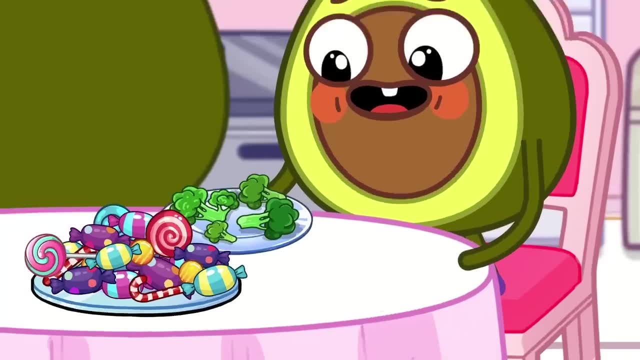 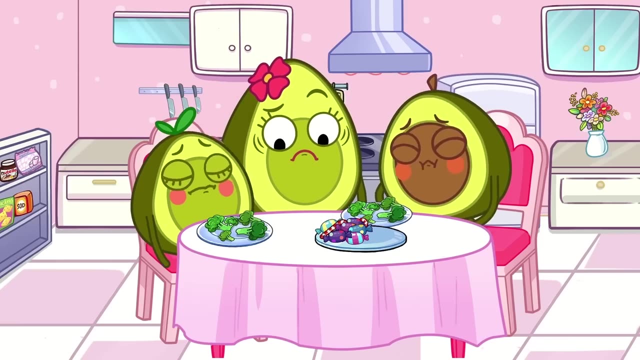 But it's time to put them away. Mommy has made lunch. What do you think Pit? He prefers sweets. Mommy is busy doing dishes. What is Pit up to? He ate half of the candy. Hey, Some of those were for Penny. 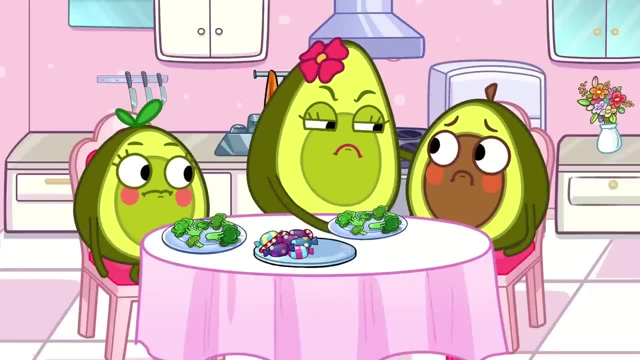 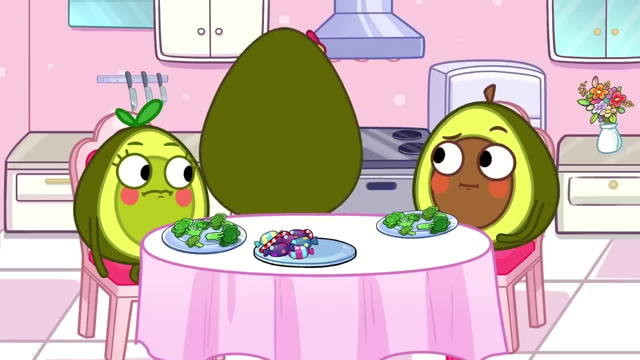 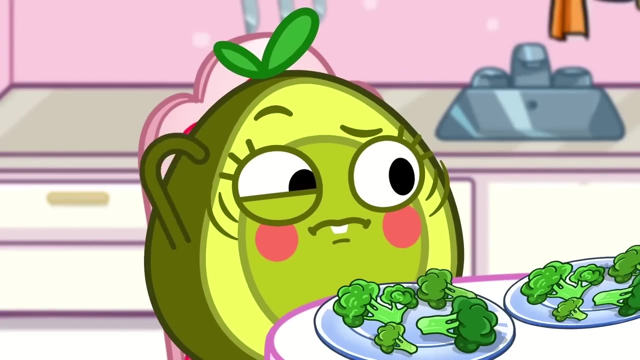 Mommy says candy is not a healthy lunch. You must always eat your vegetables first. But Pit thinks broccoli is yucky. So when Mommy goes back to the sink Pit eats all of the candy. Mommy is upset and thinks Pit needs a time out. 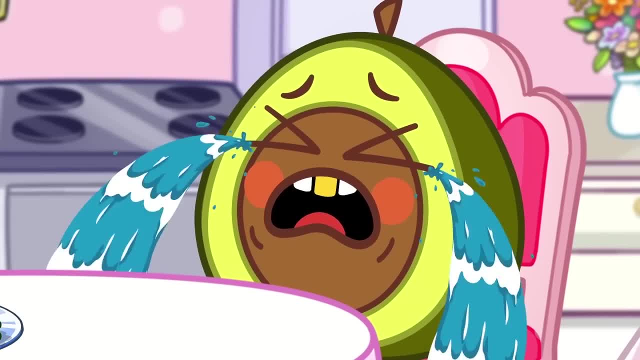 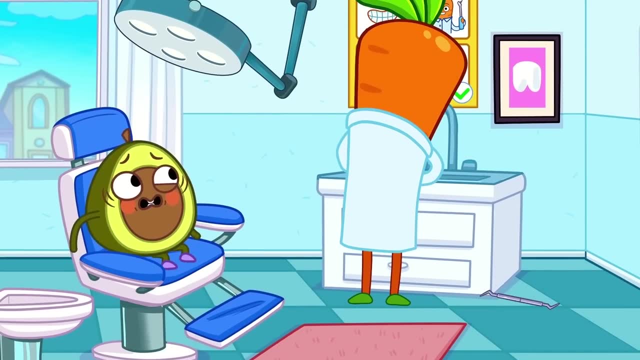 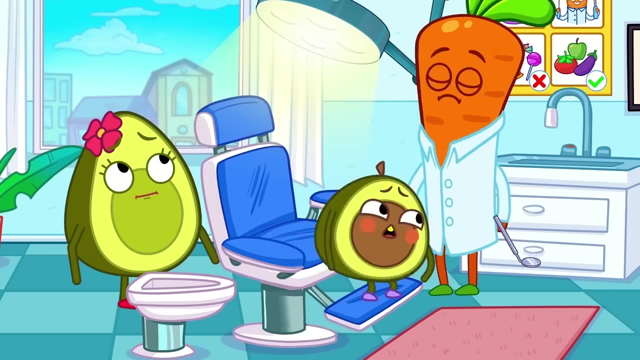 All of those sweets have given him a toothache. Pit should see the dentist right away. This is Dr Carrot's office, but Pit thinks Dr Carrot is scary. He distracts the dentist and tries to get away. Where has Pit run off to? 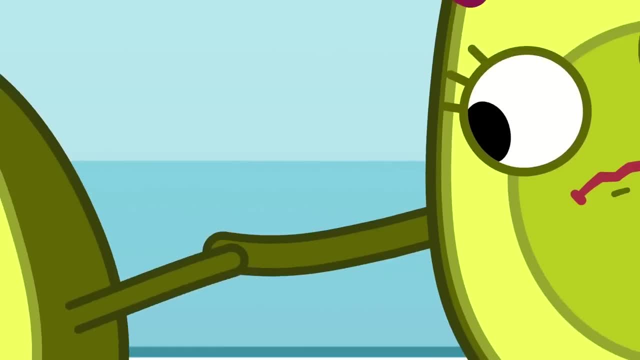 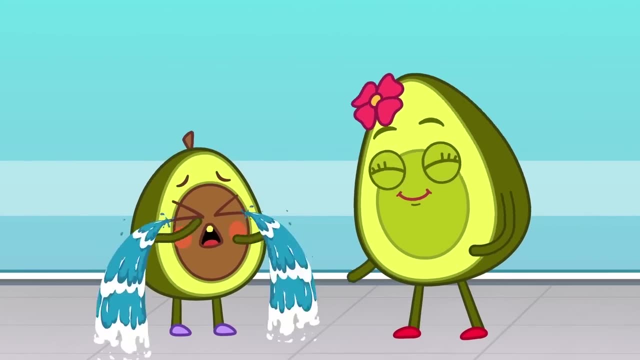 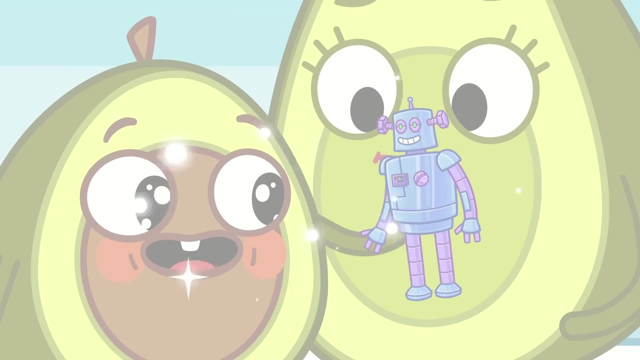 Mommy will find him. Pit, don't be afraid of the dentist, He wants to help you. Pit is still very scared. Dr Carrot has a toothache. This is an idea. Toy robot might help Pit feel brave. Pit imagines he is in a land of teeth. 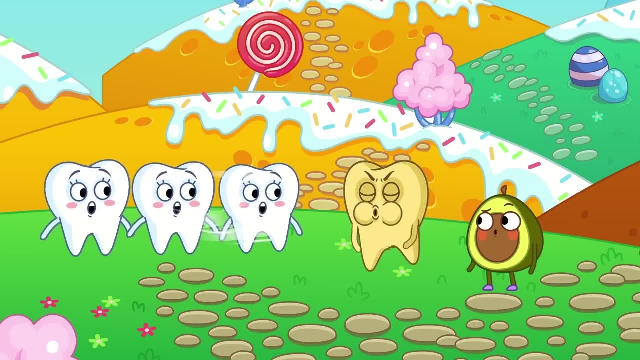 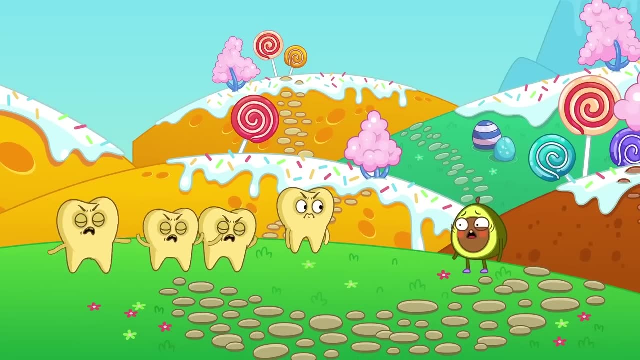 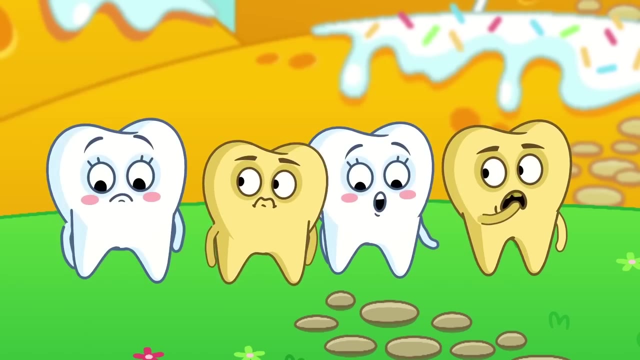 That tooth looks right. What is it up to? Oh no, Now the other teeth are rotten too. Save Pit Dr Carrot and his robot. of course, Toothpaste will turn bad teeth into good ones. Now it's robot's turn. 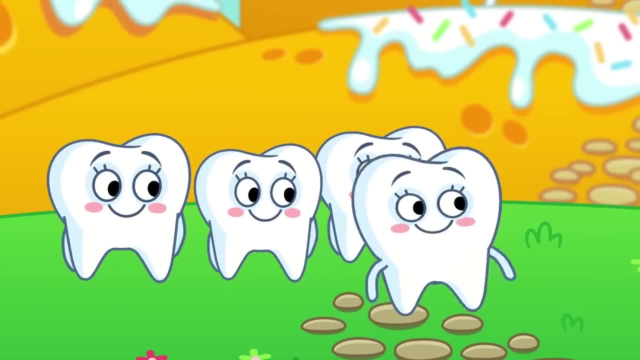 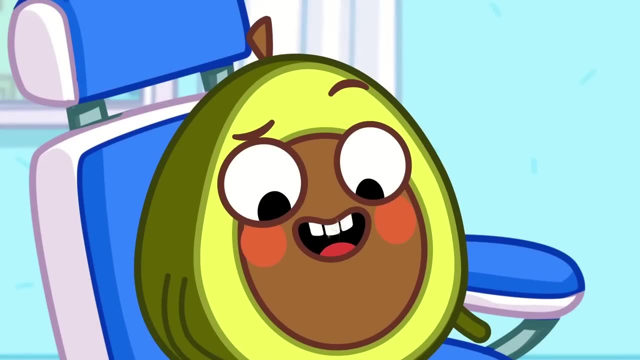 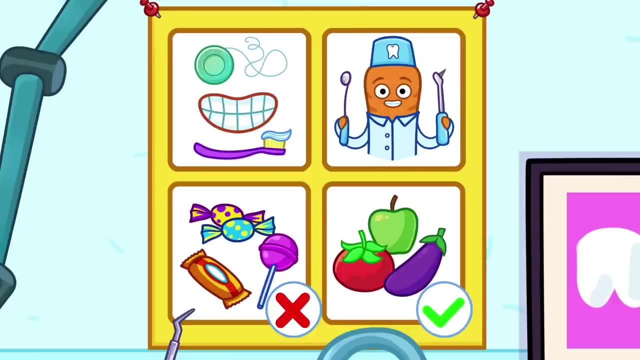 Now the teeth are happy again. Yay, Thank you, Dr Carrot. All done And look, Pit's toothache is gone. Remember these simple rules: Brush and floss your teeth. Eat only healthy snacks. Visit a dentist for check-up. 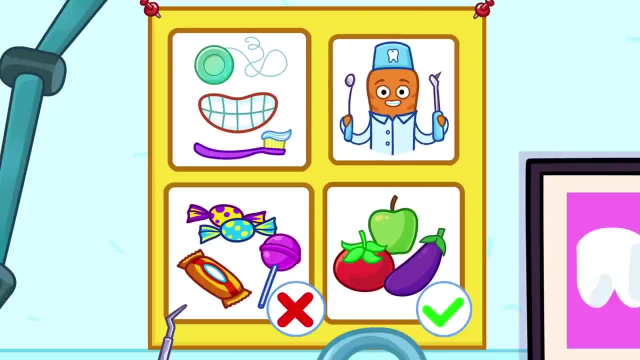 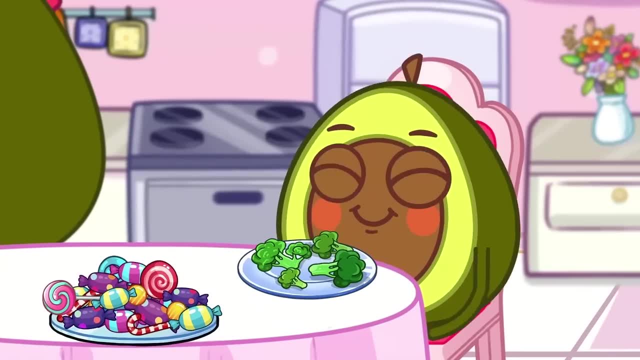 Let's see if Pit has learned his lesson. Remember to brush and floss your teeth. Eat only healthy snacks. Visit a dentist for check-up. Let's see if Pit has learned his lesson. Remember what the dentist said. Good choice, Pit. 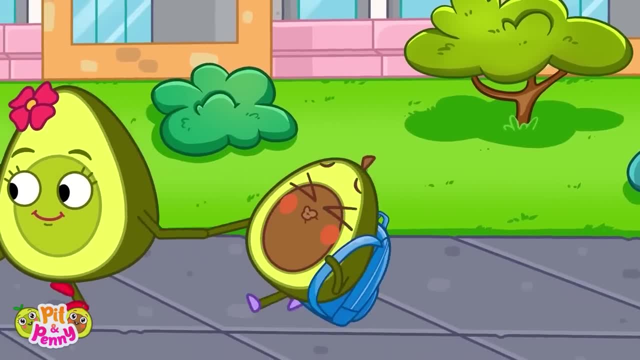 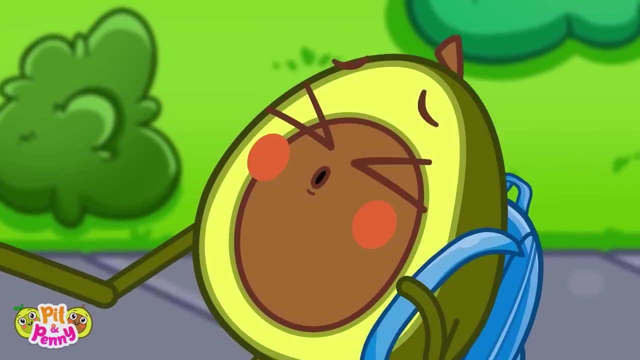 It's the first day of school, But Pit doesn't want to go. But Pit doesn't want to go. What's the matter, Pit? What's the matter, Pit? Mommy, let's go home. Pit thinks school is scary. 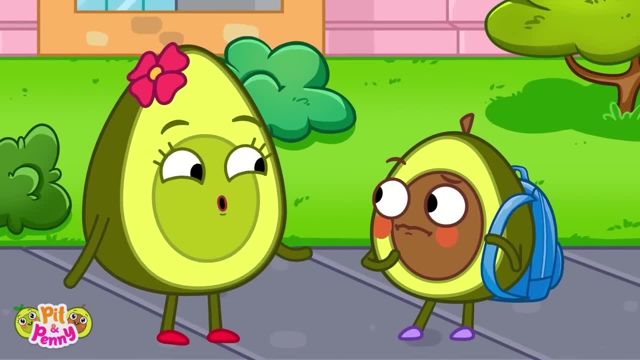 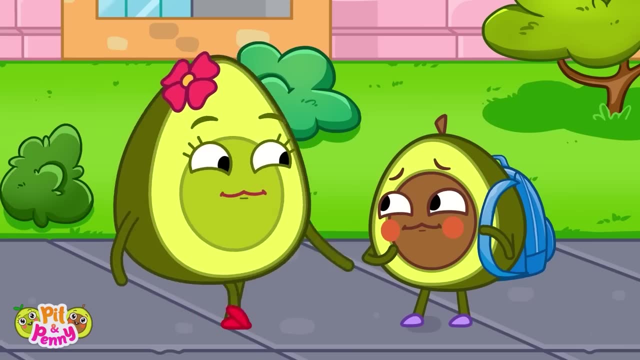 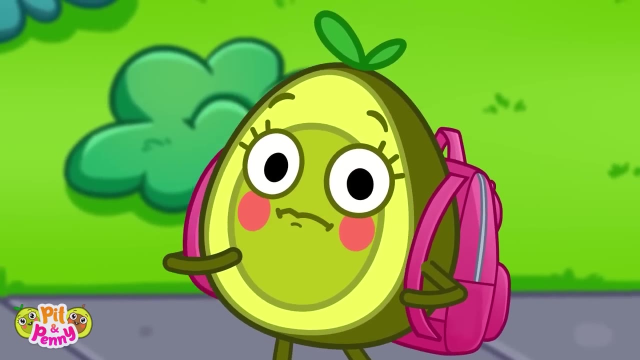 Pit thinks school is scary. The first day of school is always exciting. The first day of school is always exciting. The first day of school is always exciting. Are you ready, Pit? Are you ready, Pit? What's wrong, Penny? 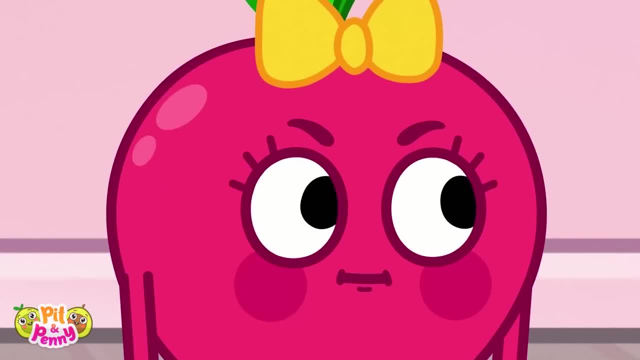 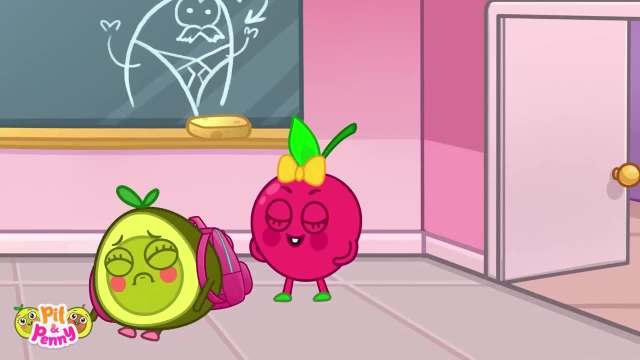 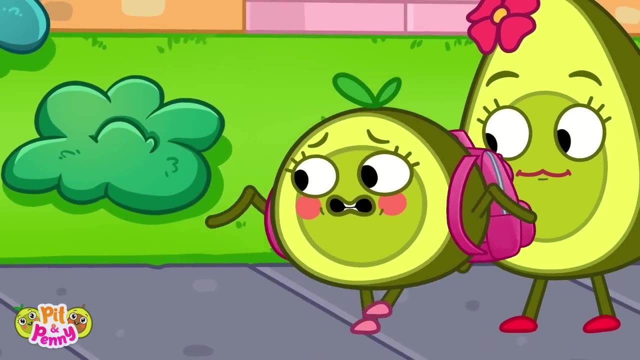 What's wrong? Penny, Watch out. That wasn't very nice. That wasn't very nice. Ow, Oh, Penny's afraid she'll get picked on. Oh, Penny's afraid she'll get picked on. Penny, don't be afraid. 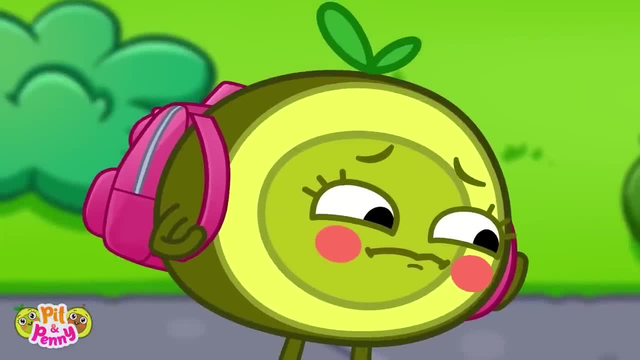 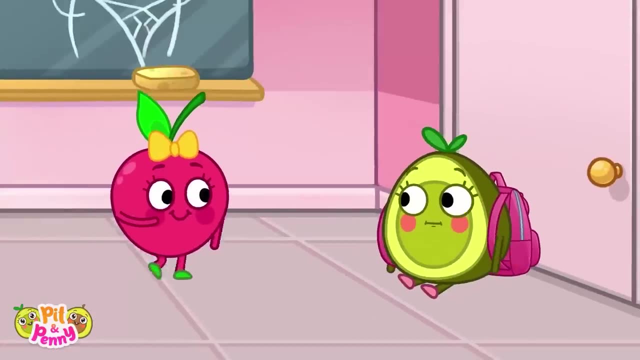 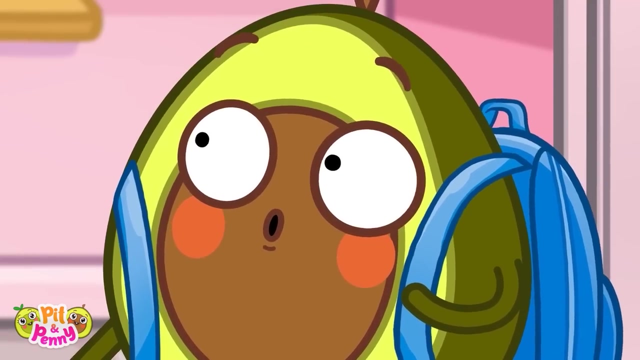 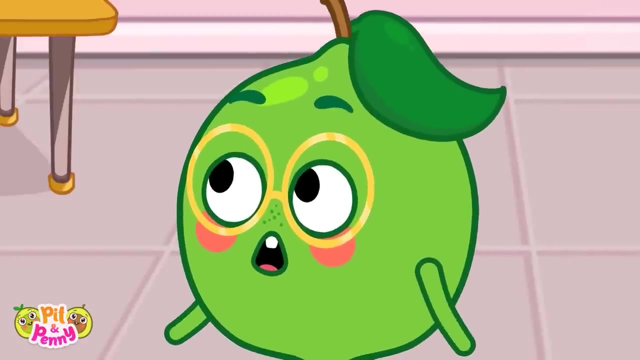 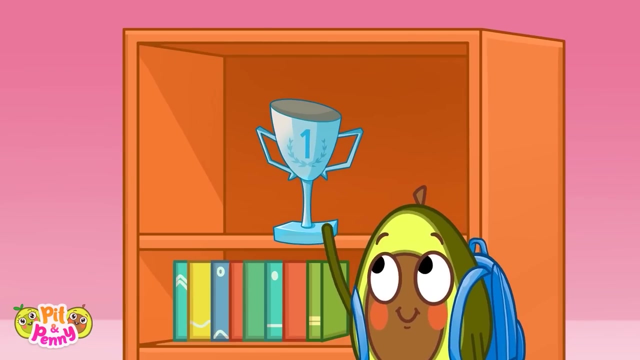 School will be fun, be fun. Oh, Poor Penny. Oh, But someone's there to help. But someone's there to help. Oh, Oh, no, The trophy is going to fall. Good catch Pit. Do you want to play with us? 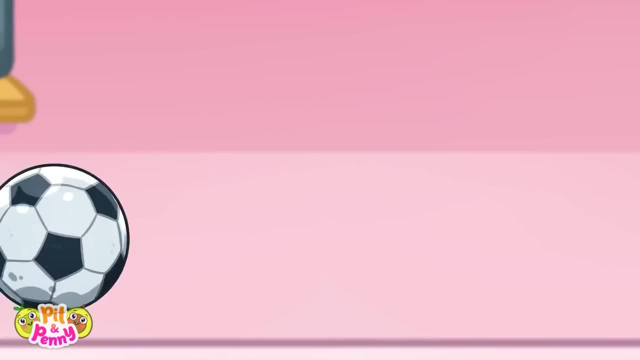 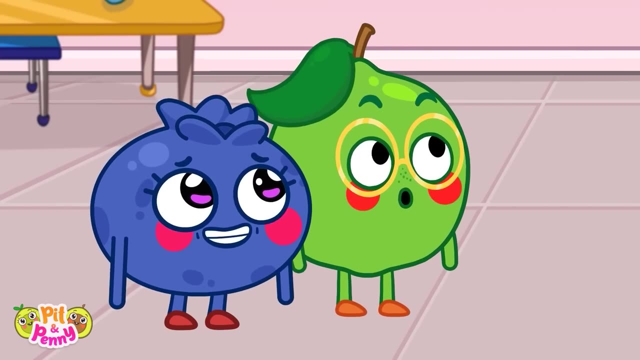 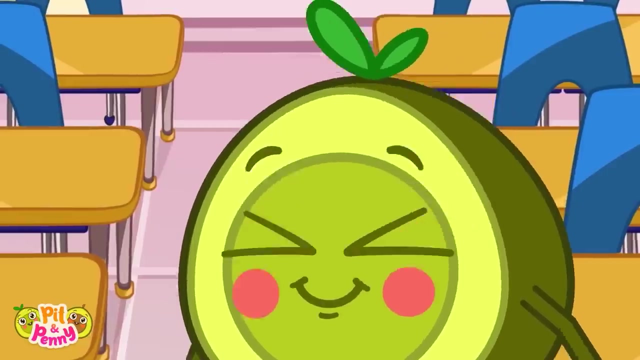 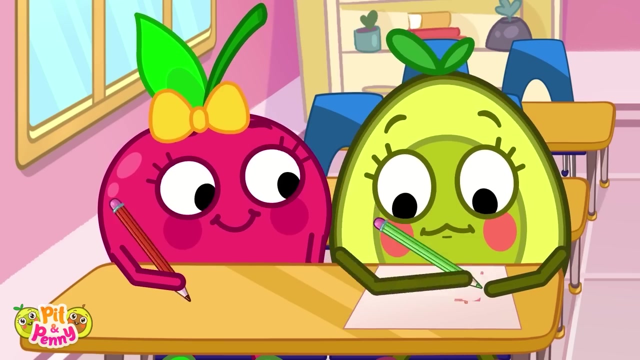 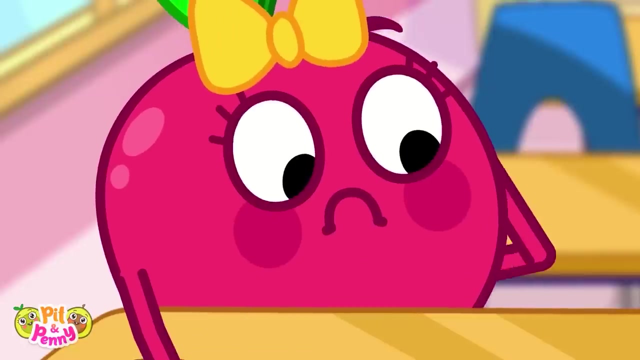 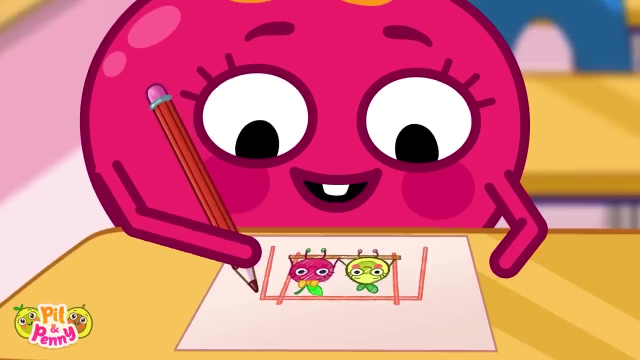 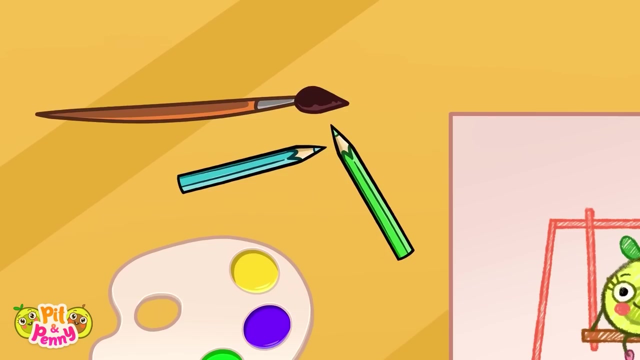 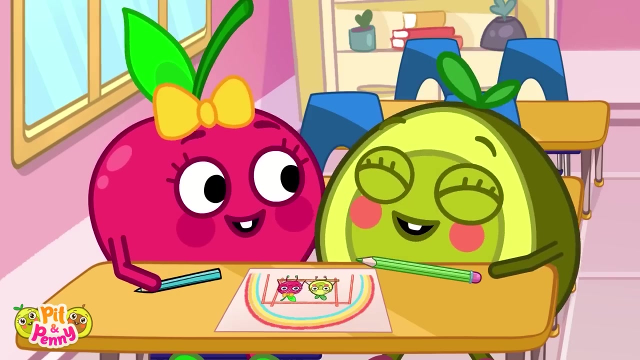 Playing ball inside is not a good idea. You can only play the ball outside And now draw how you play with friends. What will Penny draw? Something's missing, but what A friend. What a perfect picture. Pit, you can't play teeter-totter by yourself. 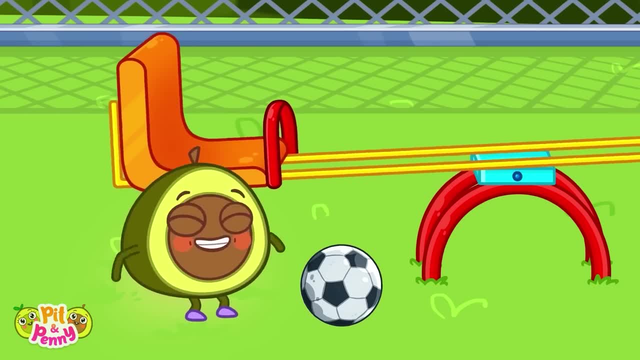 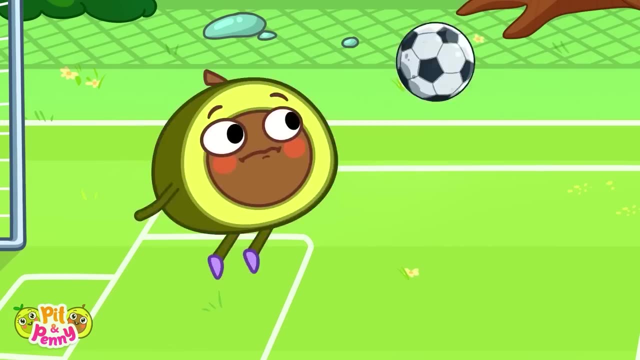 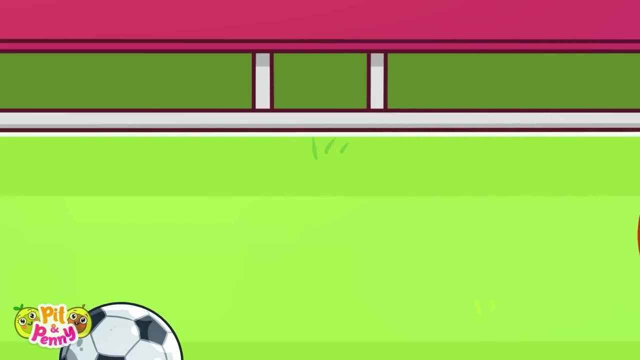 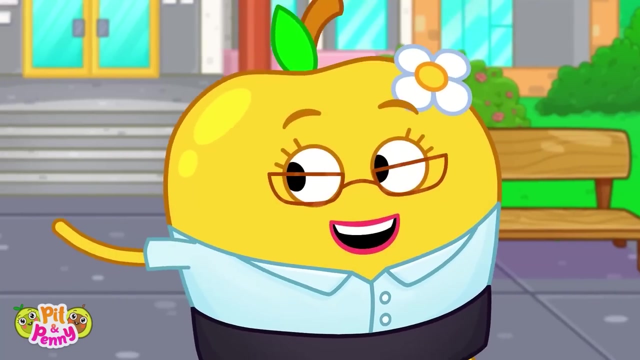 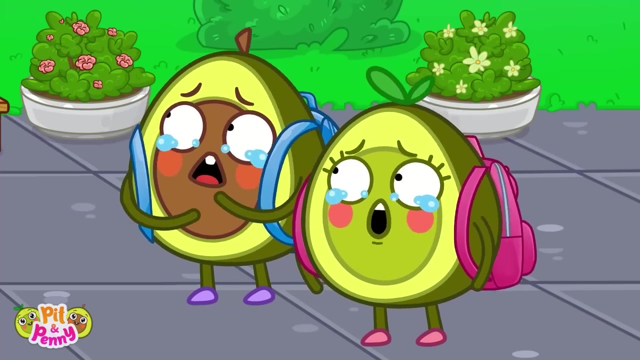 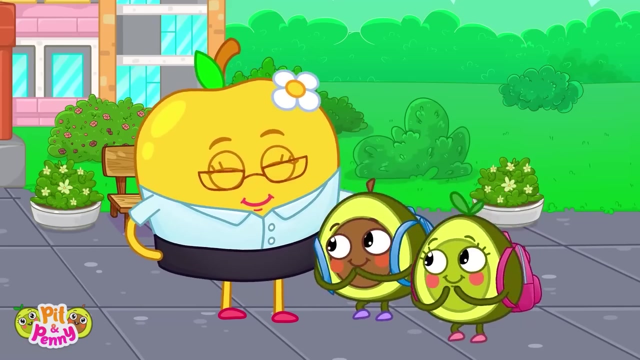 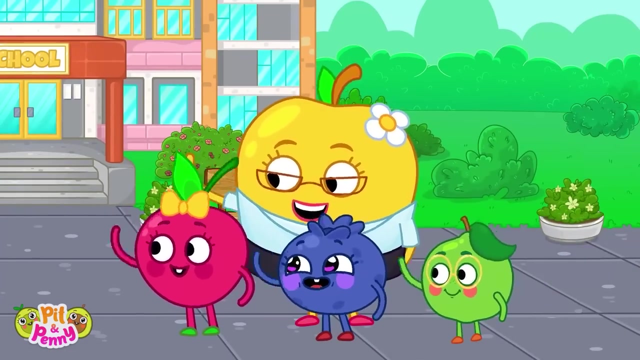 Let's play football. Here comes the ball Pit. Penny, your mama's here Now. what's wrong? We don't want to go home. Don't cry. Tomorrow you will go to school again. Bye Pit, Bye Penny. 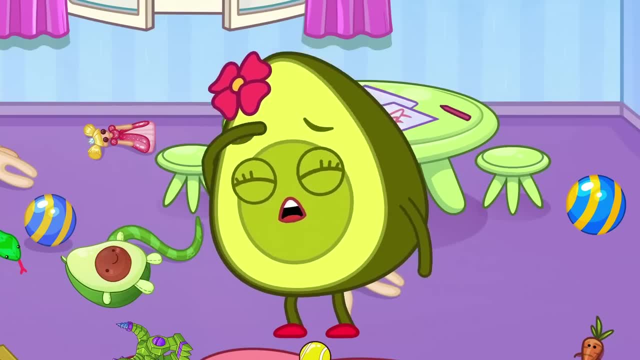 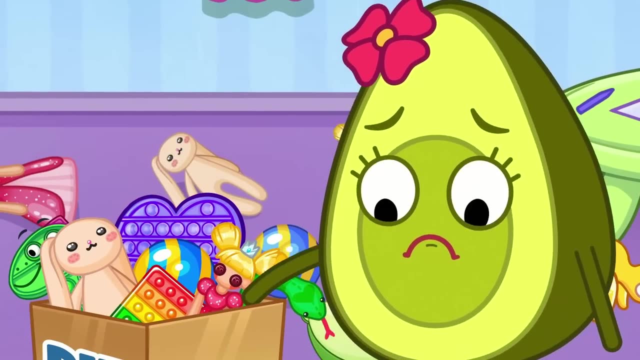 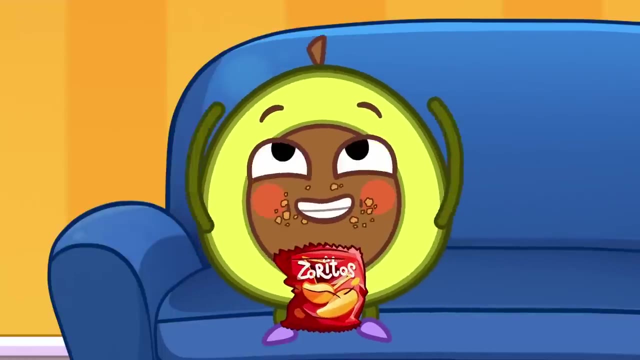 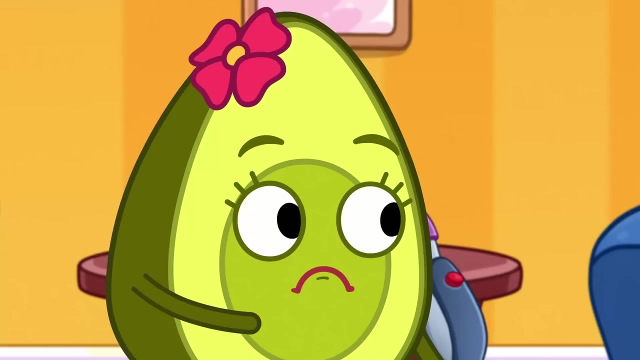 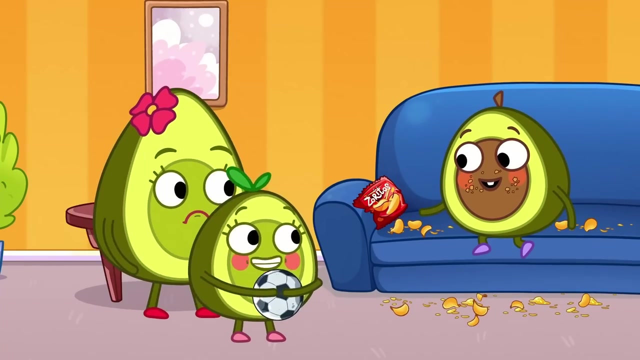 I'll find it Pit. Just a second. Hmm, These chips are delicious. No, no, no. Oops, Missed some Pit. It's just a little mess. Let's go play. Okay, Mommy will clean this up. 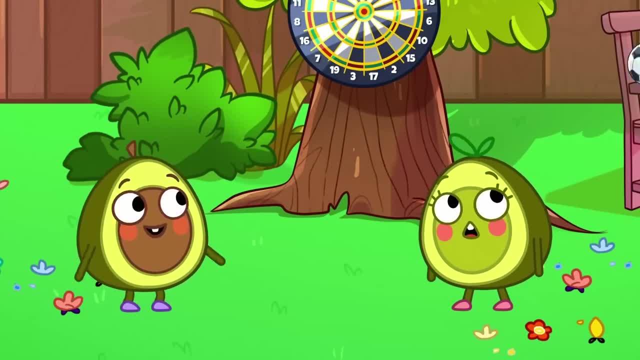 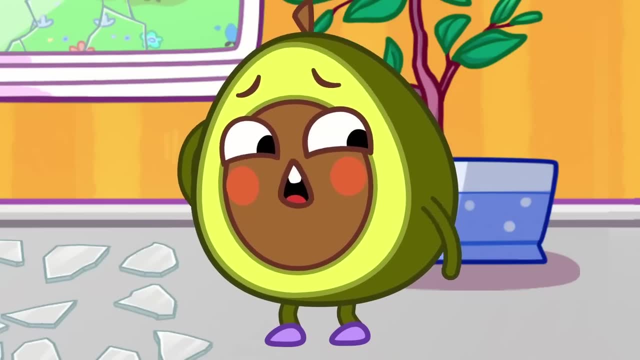 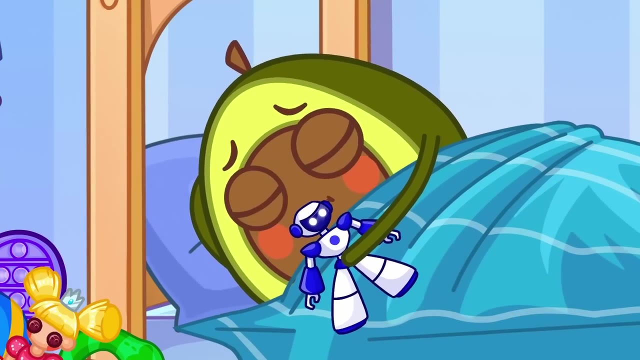 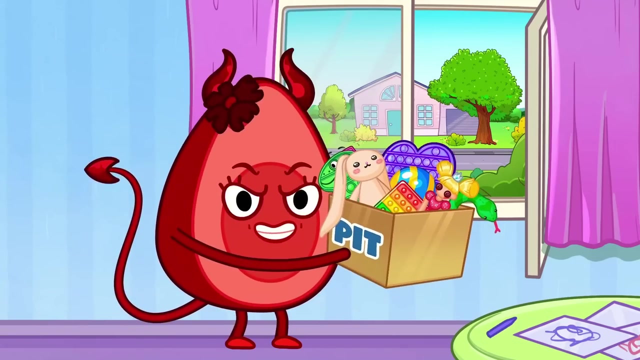 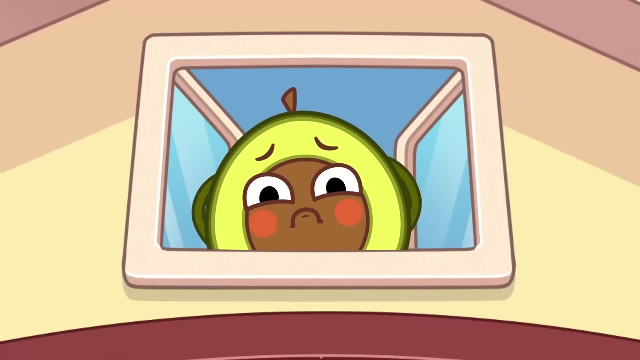 Catch. You won't catch this. Oh, Huh, Pit Whoops. Sorry, Time for bed, Mr Robot. Ah, Sweet dreams. What happened to Mommy? Oh, no, My toys. No, Mommy, You'll make a mess. 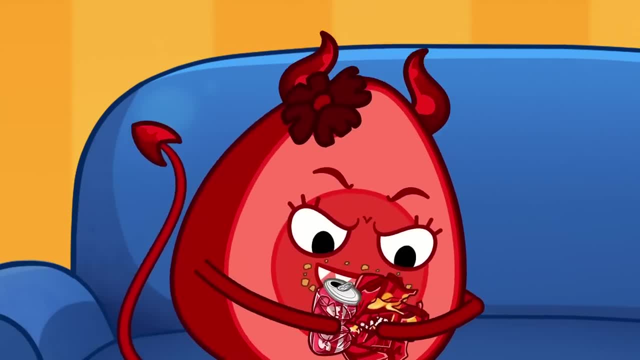 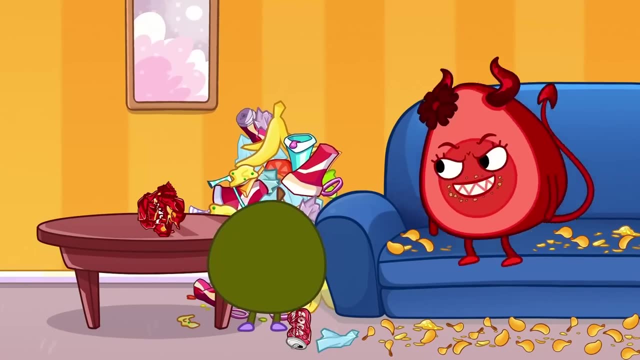 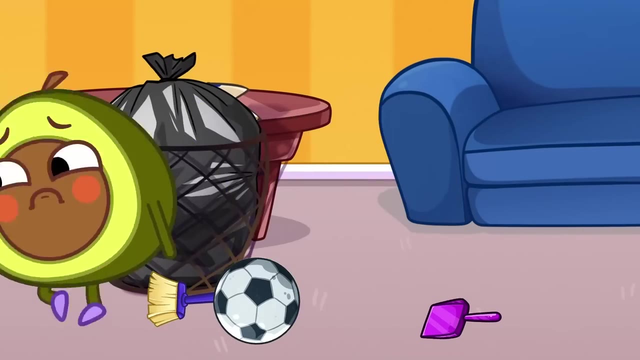 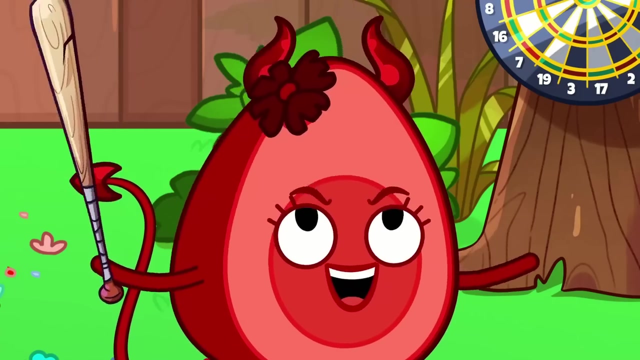 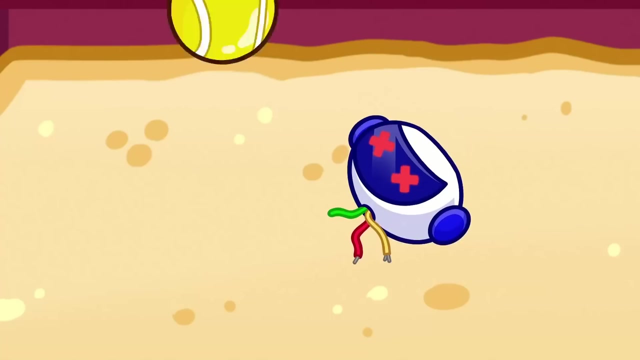 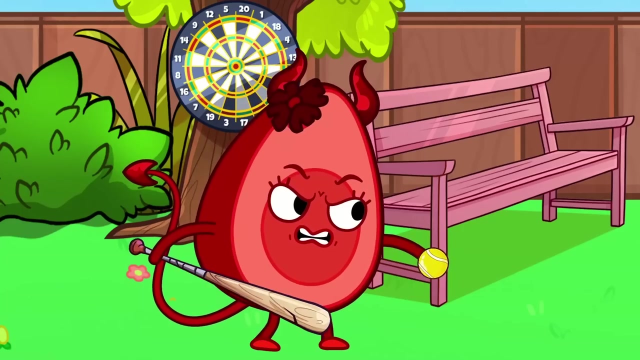 Mommy's a demon. I'll have to clean up. Phew All done. Oh no, I better check outside Now. the window is broken. No, Don't do it. That was my favorite toy. It's Angel Mommy. 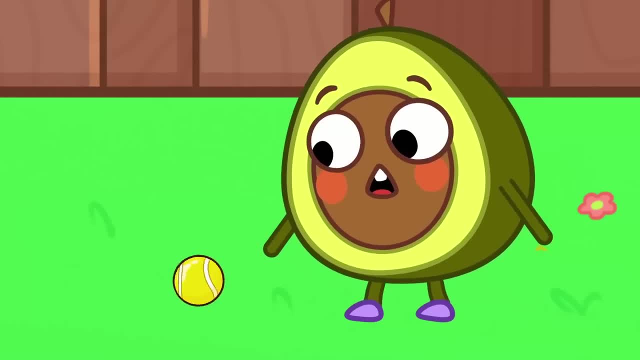 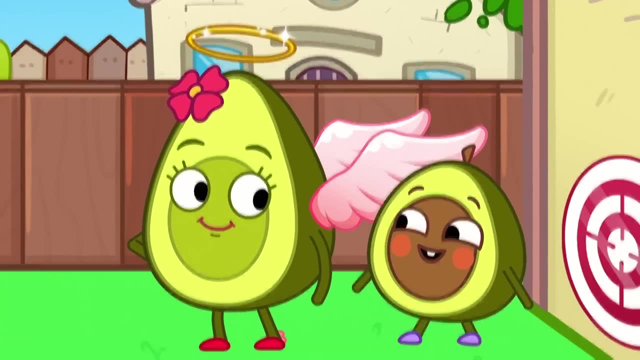 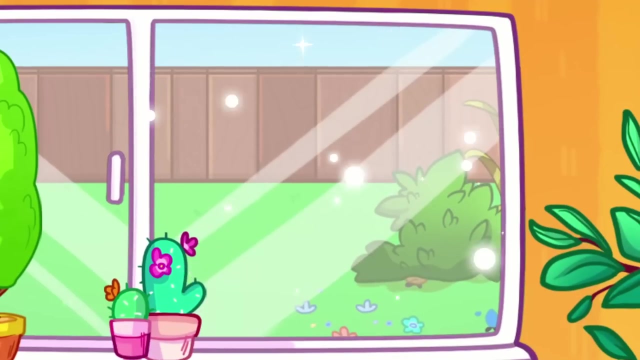 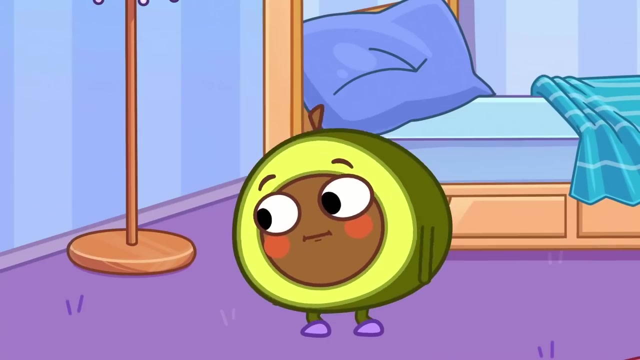 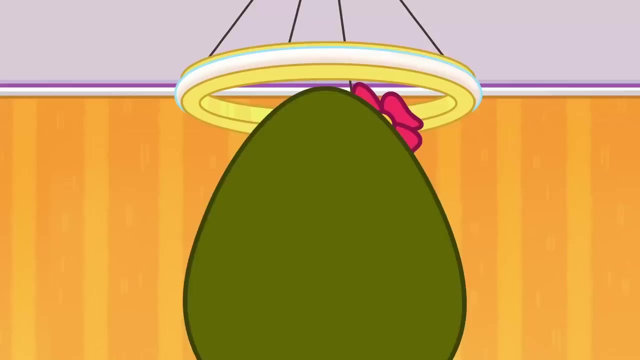 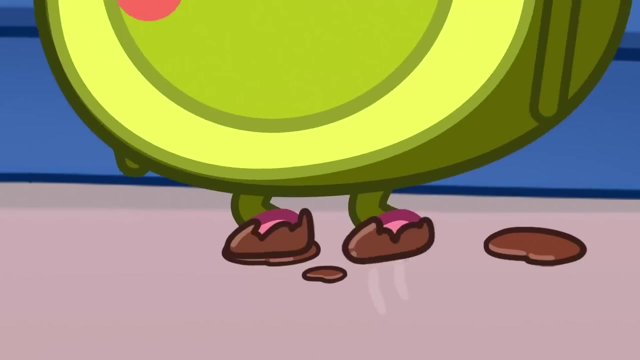 Help. Angel Mommy. Demon Mommy is gone, But what about the broken window? All fixed, Yay, Yay, Hmm, I wonder what that noise is. What's going on? Mommy is an angel. Penny, You're making a mess. 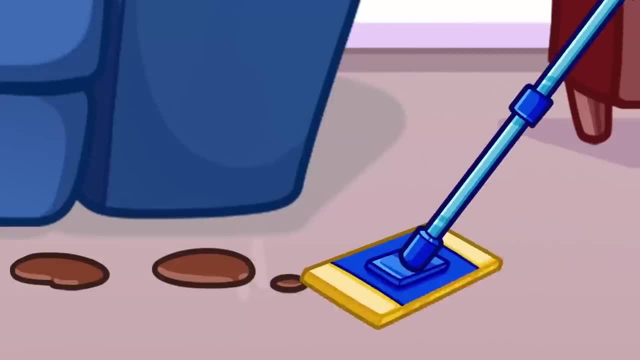 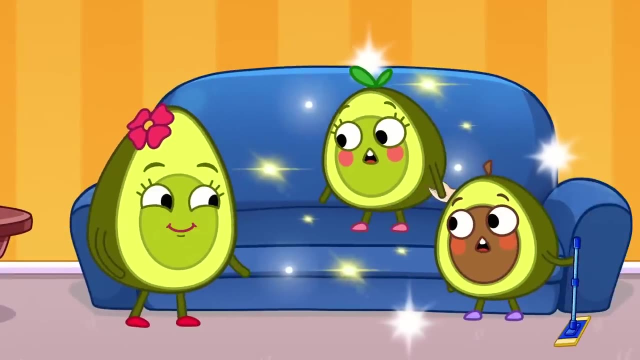 Oops, Sorry, Let's clean up so Mommy doesn't have to. Yeah, Oh, Well done. Well done, kids, You're welcome, Hii-hii-hii, Hii-hii-hii. PITT has been playing all morning. 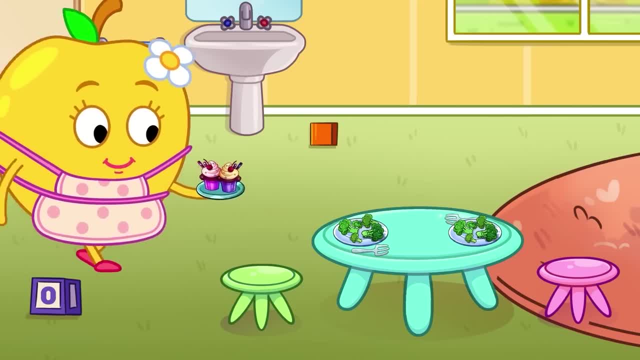 And it's almost time for lunch. PITT, PITT, PITT, PITT, PITT, PITT. Shouldn't Pitt do something before he eats? Put the toys away. Pitt PITT thinks Miss Apple is a monster. 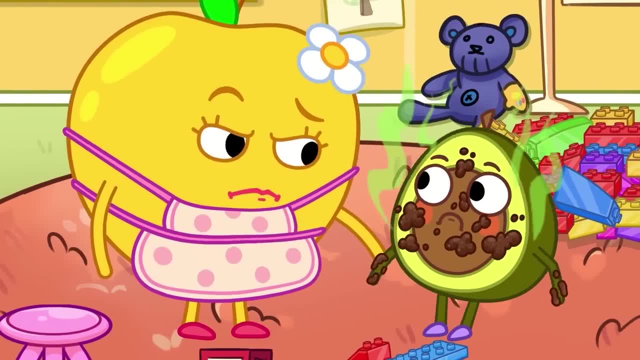 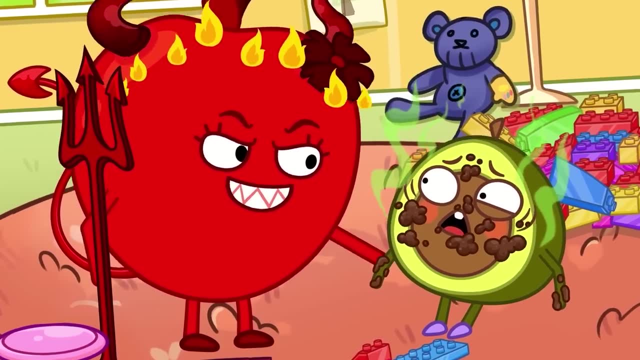 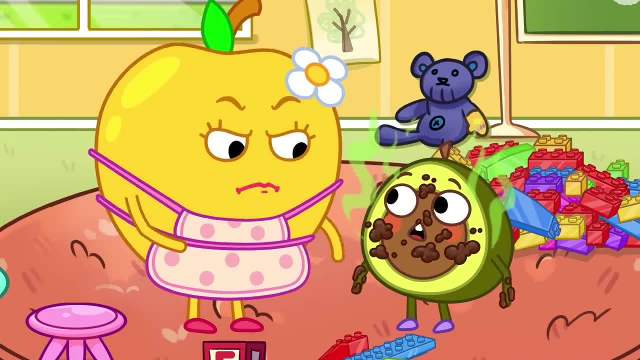 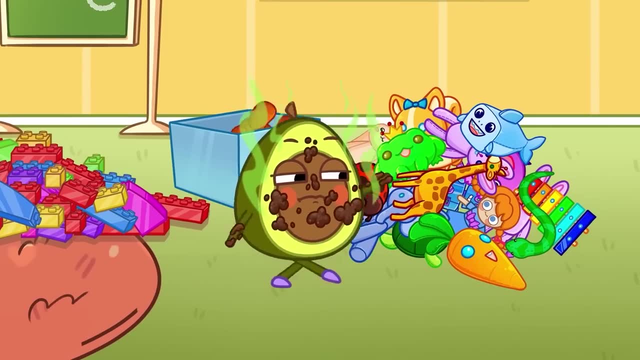 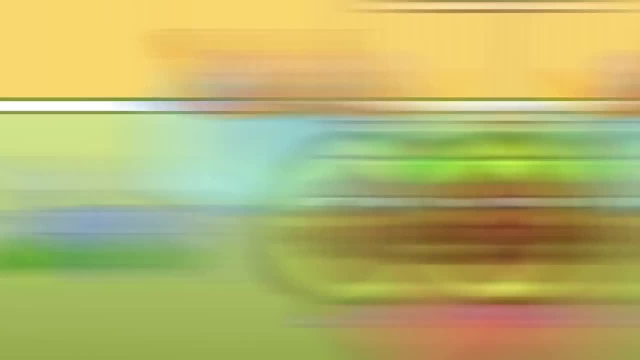 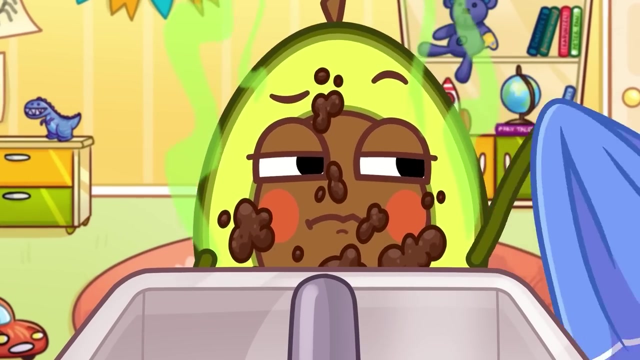 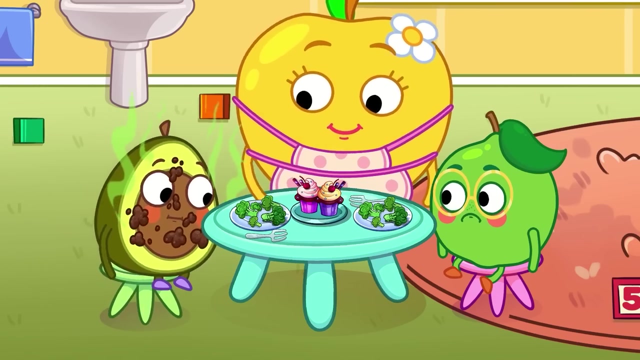 I'm so hungry, a monster And wash your hands. It's always good to clean up your mess, Pit, And it's important to wash your hands and face, But Pit isn't trying very hard. Vegetables: Pit would rather eat the cupcakes. 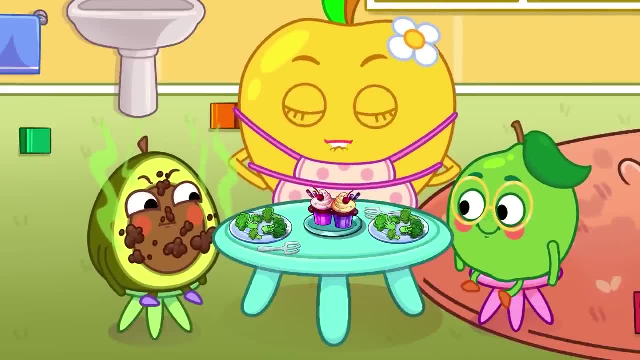 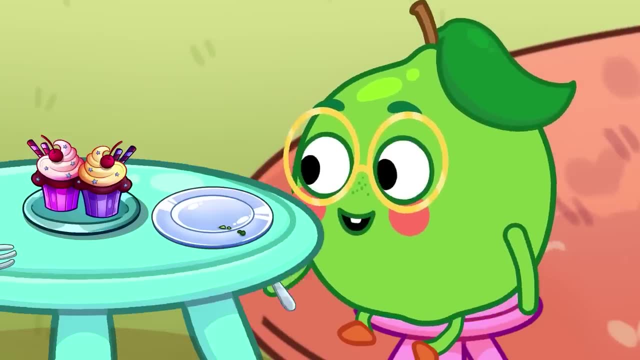 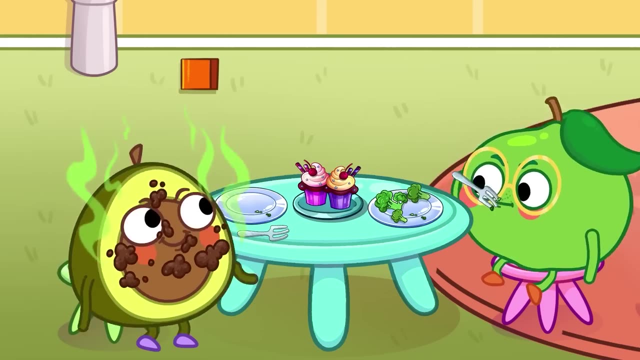 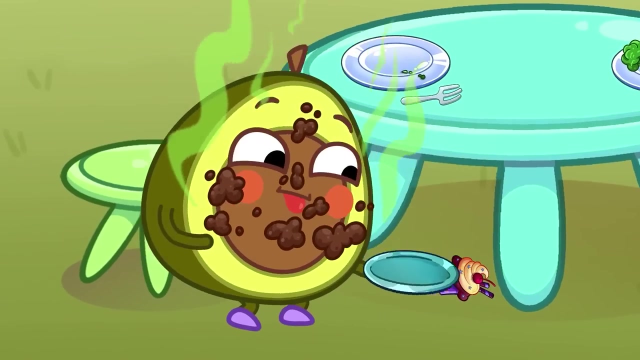 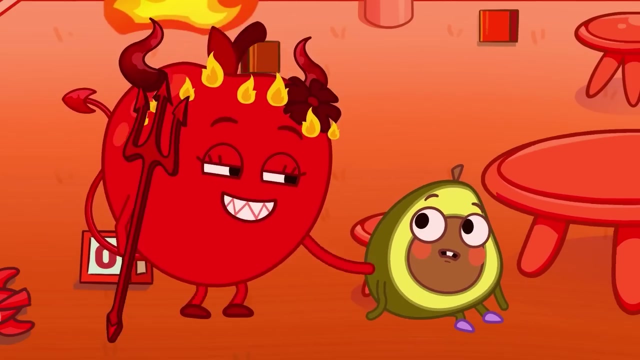 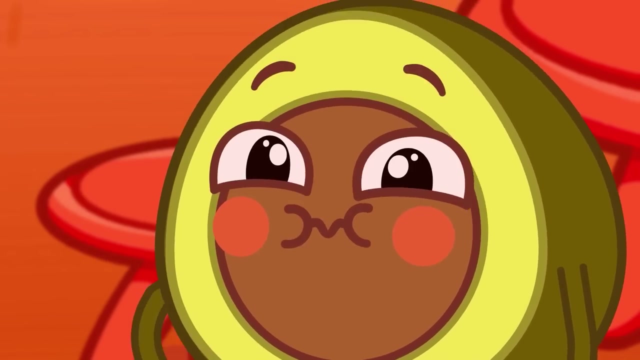 Pit, Vegetables are good for our health. See, Lime is eating his vegetables. Pit has a sneaky plan. Oh, Pit, Are you? okay, Pit, It's Miss Apple as a monster again, And she wants you to eat all the junk food you want. 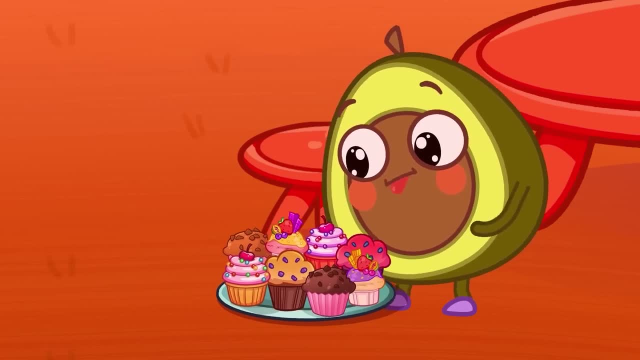 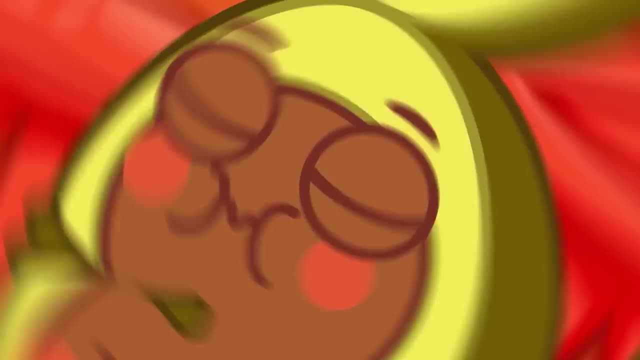 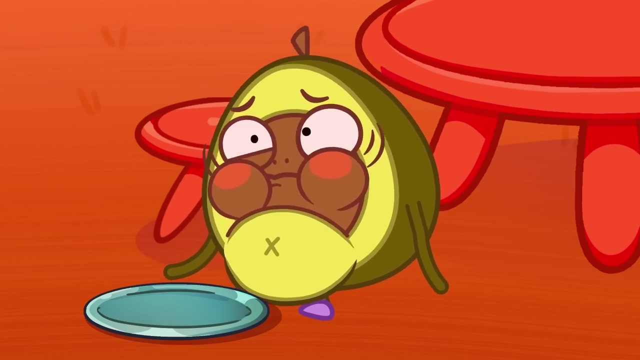 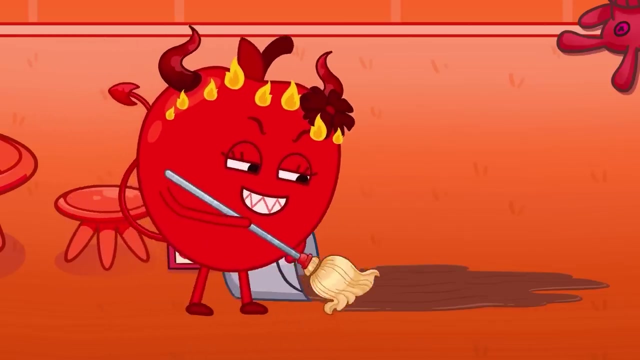 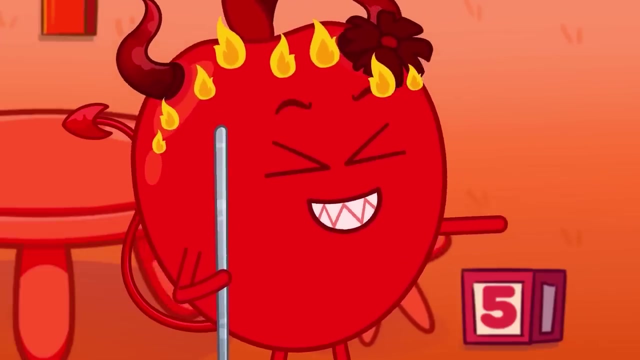 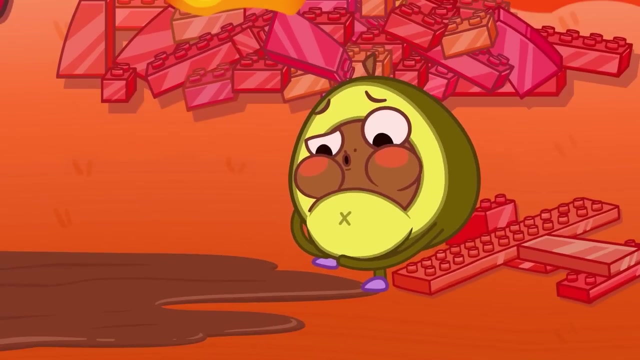 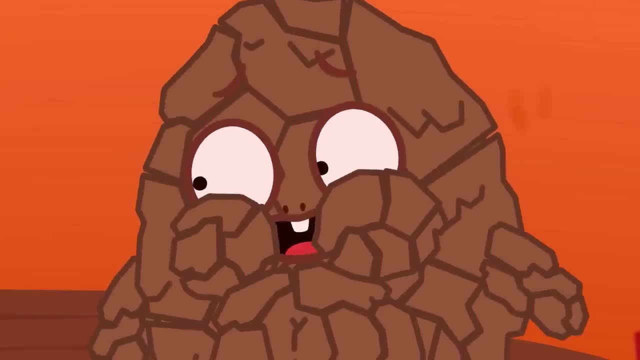 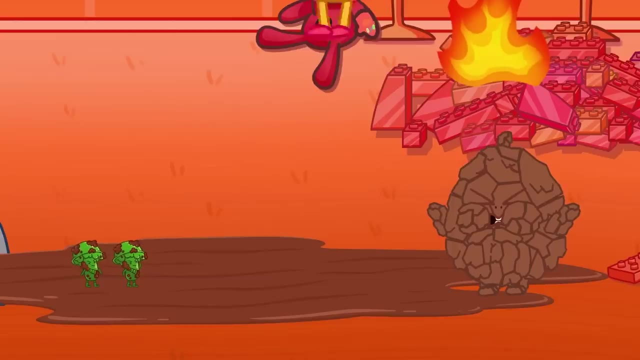 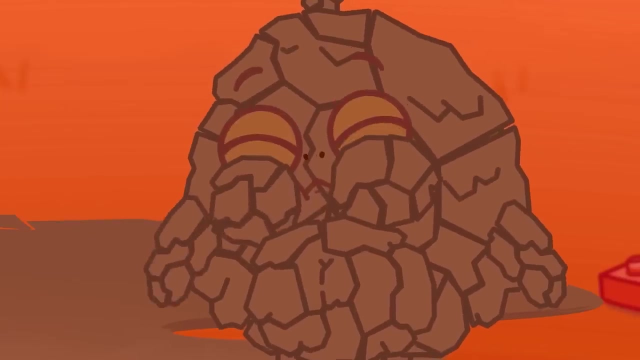 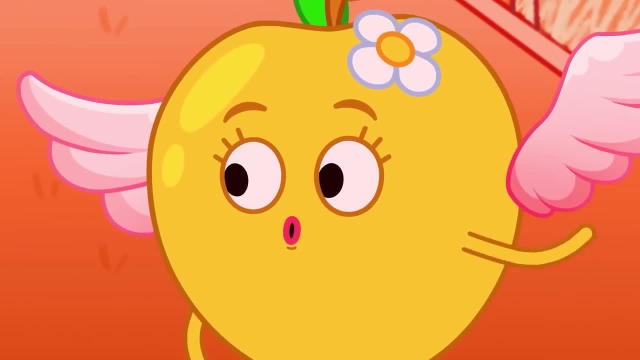 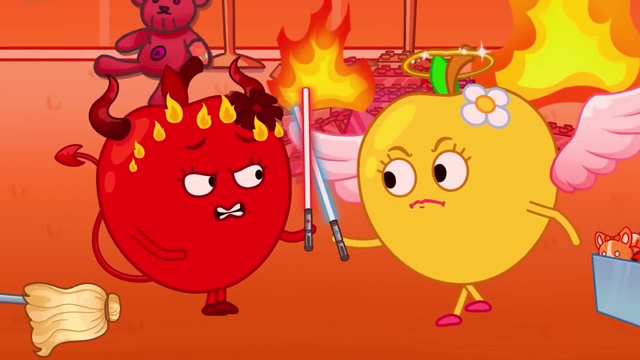 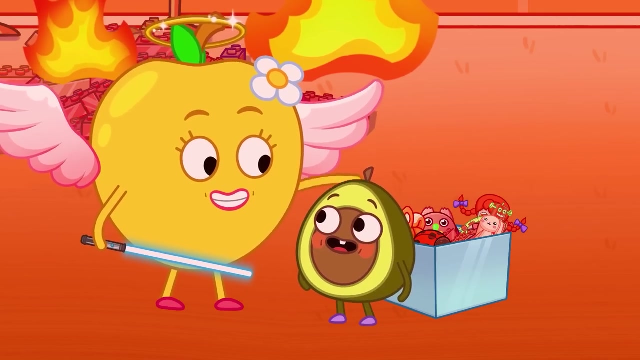 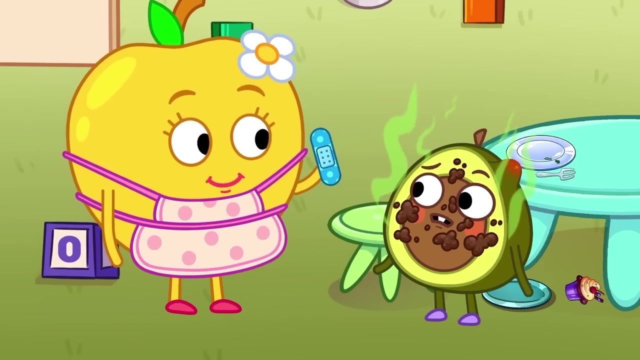 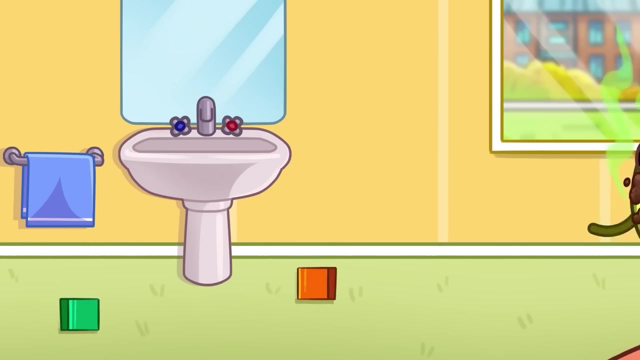 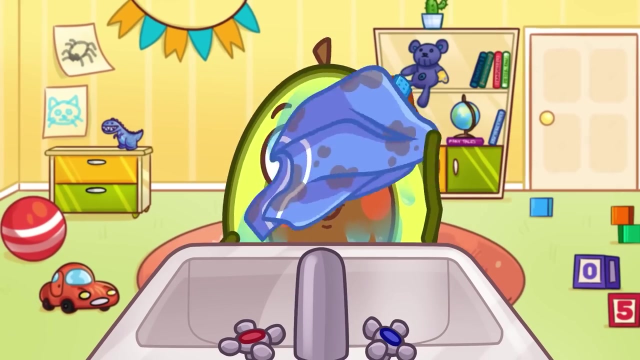 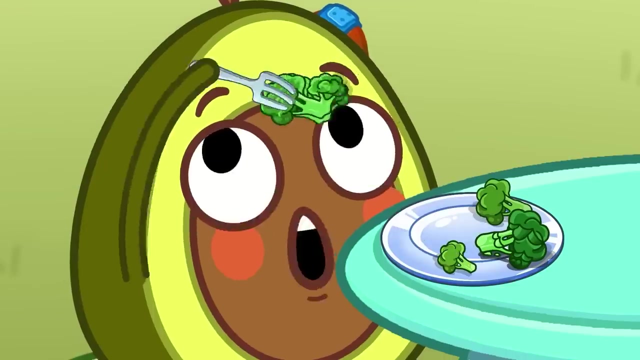 Look, Don't worry, Pit Angel. Miss Apple will deal with her. It was just a dream. Here's a bandage for your bump. Now Pit will clean up properly And wash his hands and face. He'll even eat his vegetables. 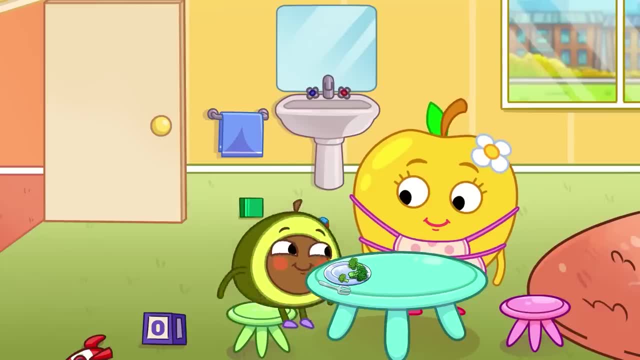 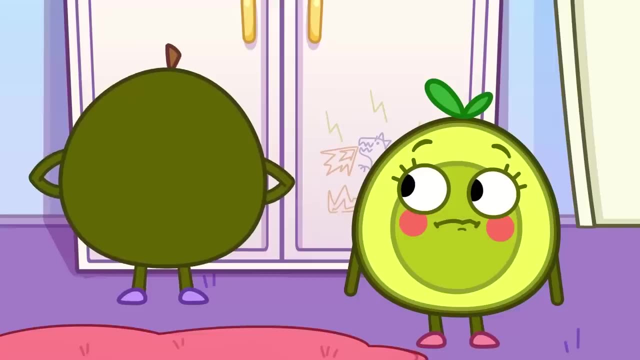 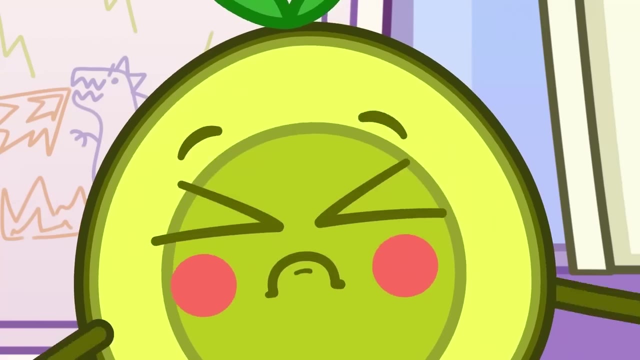 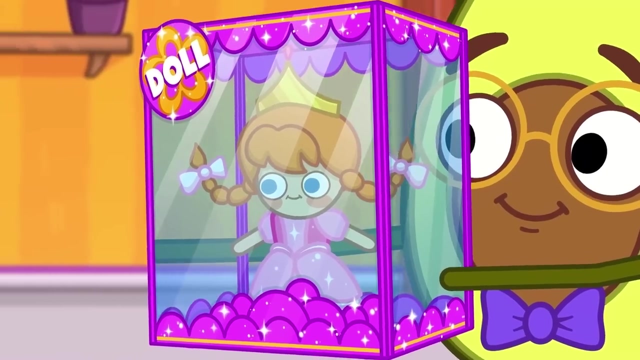 I'm sorry for my behavior. Well done, Pit. Where can I hide? Some place? Pit won't find me. I don't have much time. I've got it. I'll leave a trail for Pit to follow. What a pretty doll. 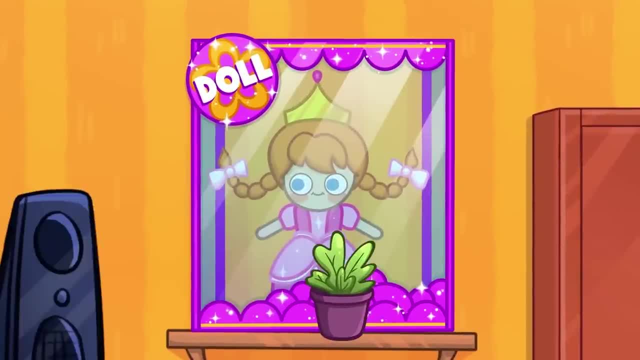 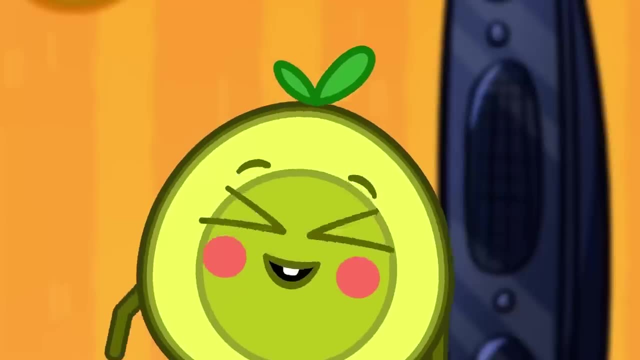 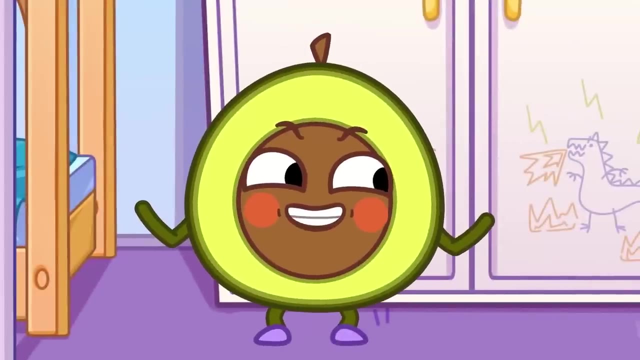 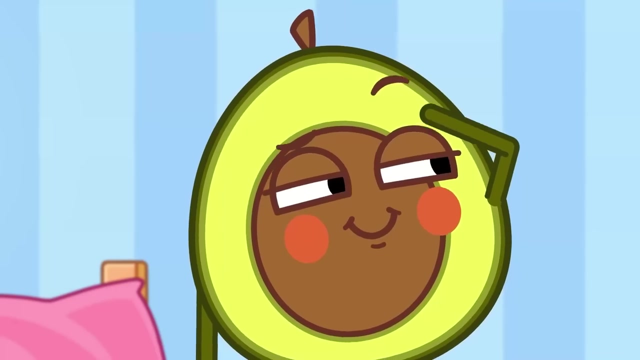 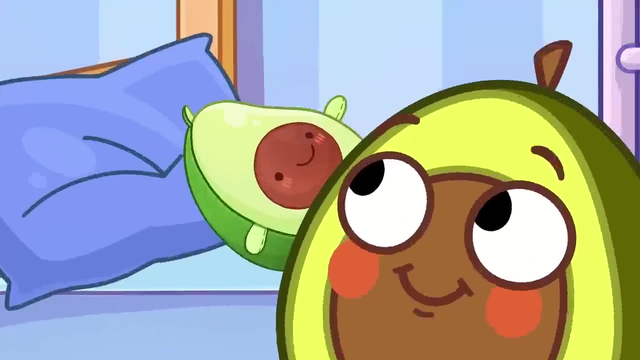 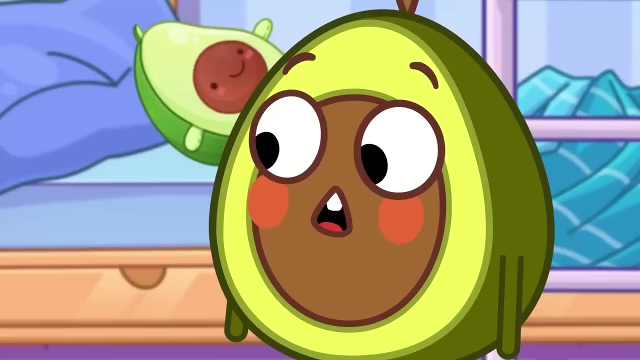 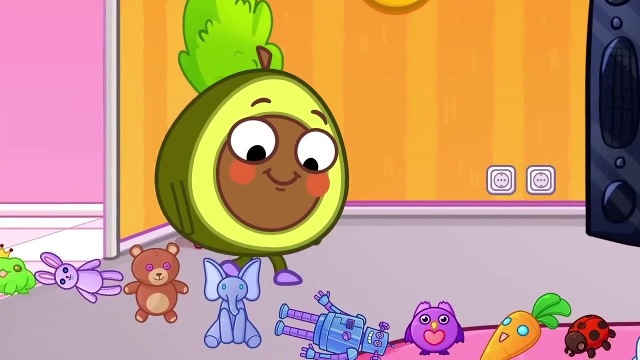 What's Daddy up to? He's hiding the doll on the shelf. That gives me an idea. Nine, ten, I bet Pit won't find me. Am I in the bed? Nope, Next he'll follow my trail of toys, Uh-oh. 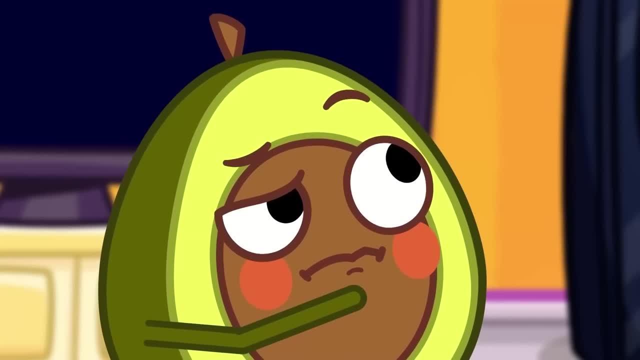 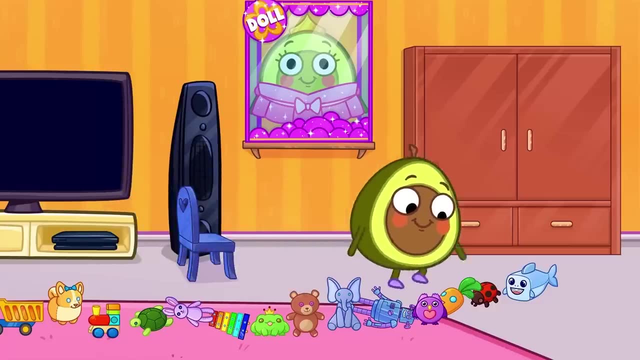 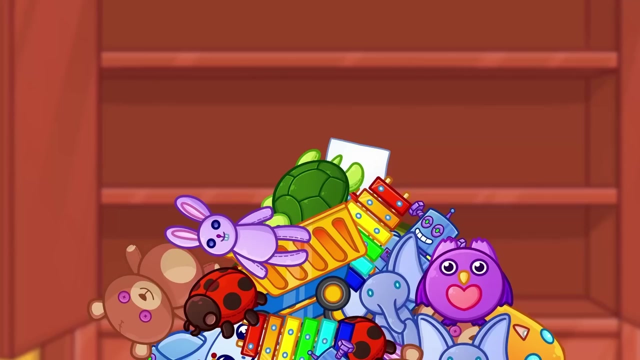 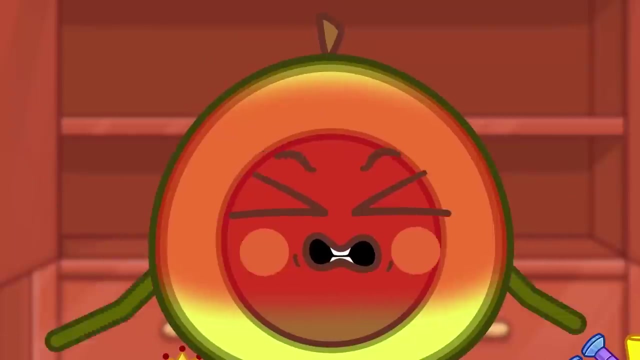 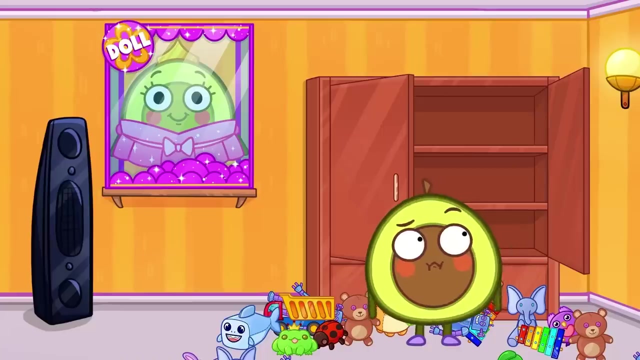 I need to stay perfectly. still, Has he spotted me? Pit thinks I'm in the cupboard. I'm not, But I left a note. Na-na, You can't find me. I think he heard me Now. Pit thinks I snuck out the door. 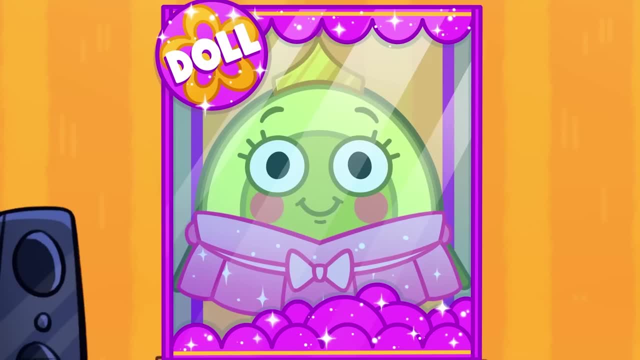 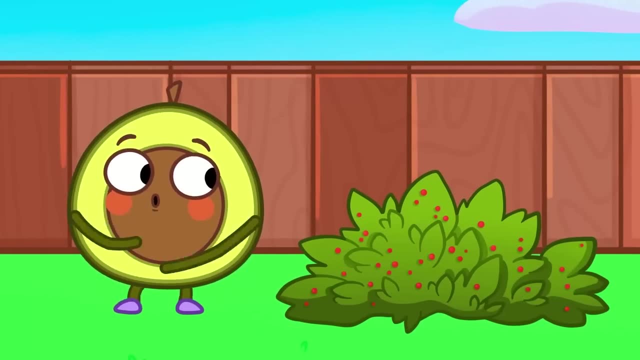 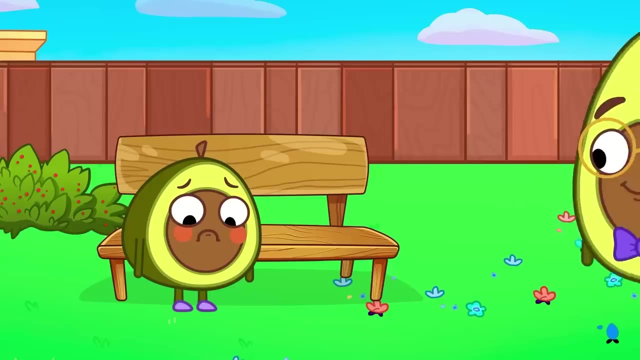 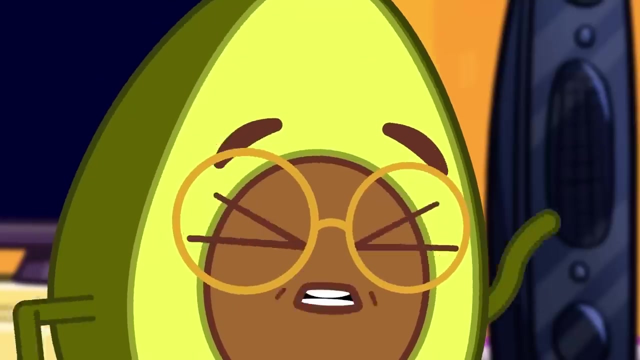 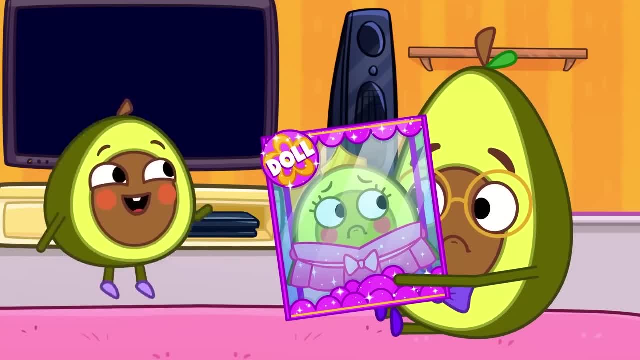 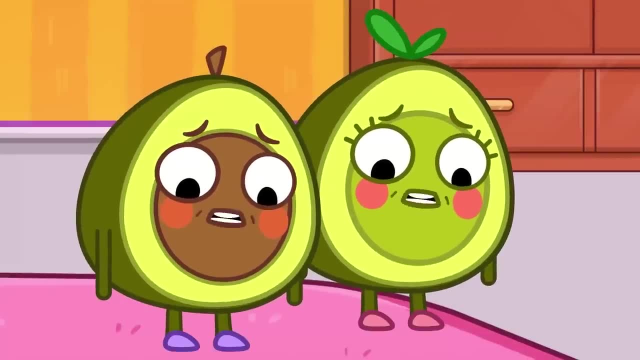 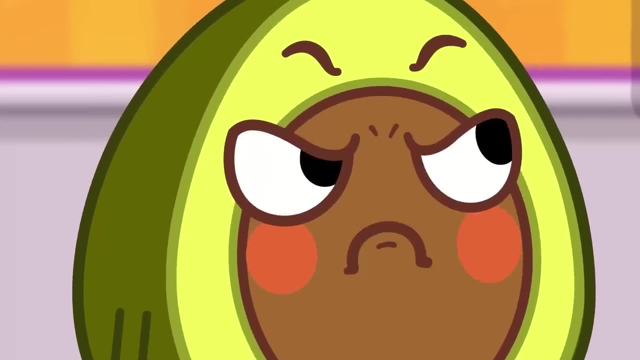 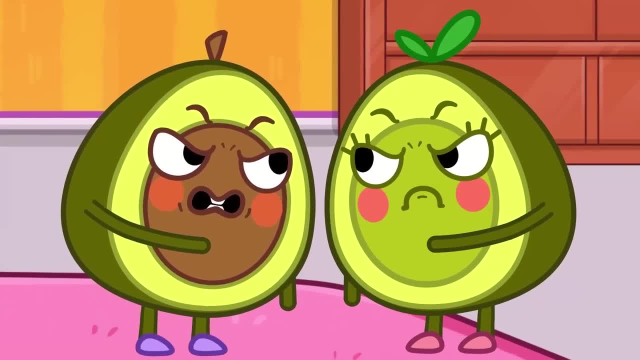 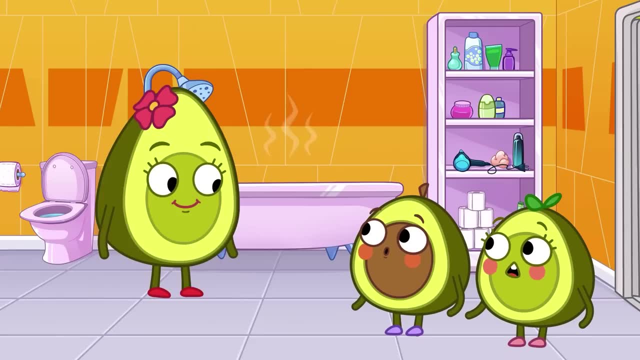 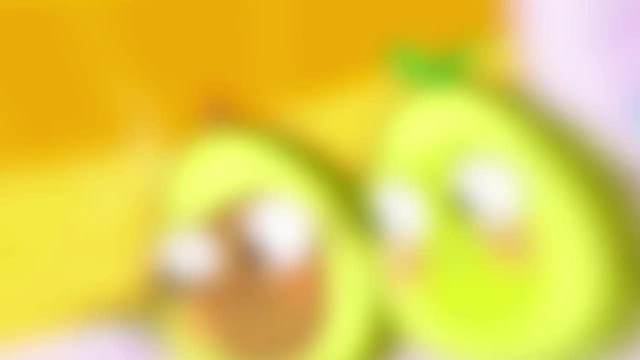 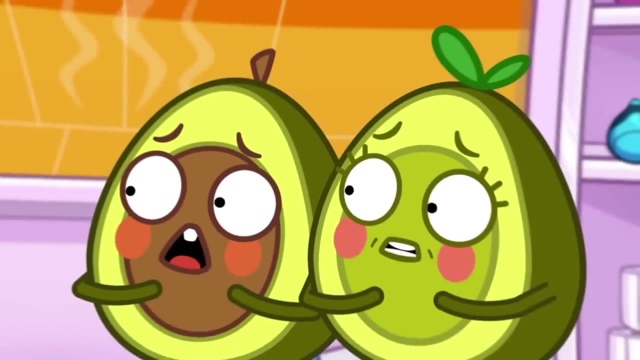 No, I won. Who won, Daddy He-he? Oh Pùtty, Look, Look, Look. Pit and Penny, it's time for your bath. They think the water is too hot. They don't want a bath today. 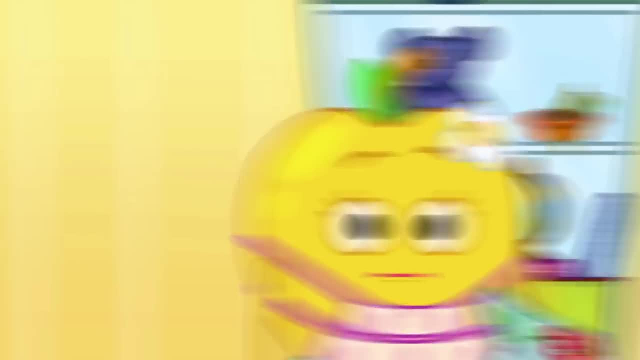 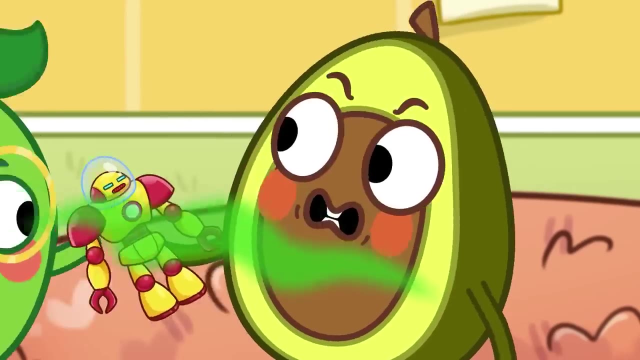 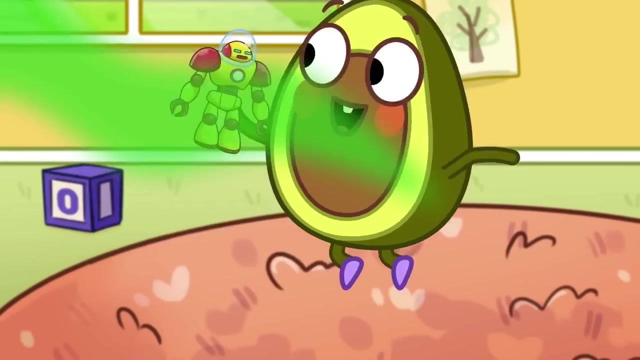 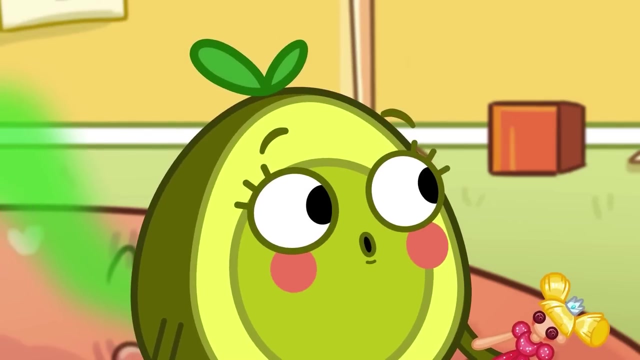 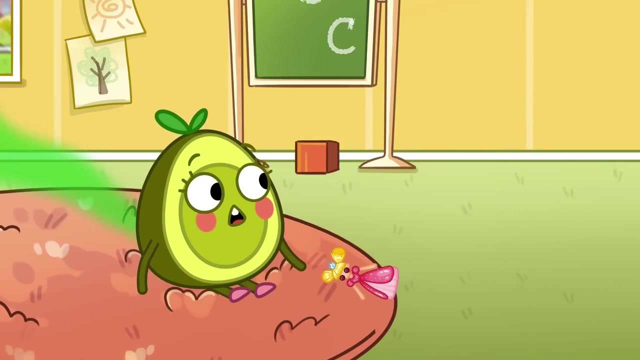 Sorry, Miss Apple, Pit and Penny haven't bathed. Pit doesn't want to share with Lime And Lime thinks Pit is too smelly. Will Penny share with Cherry? Oh no, Penny's doll is a little smelly. Let's give the doll a bath. 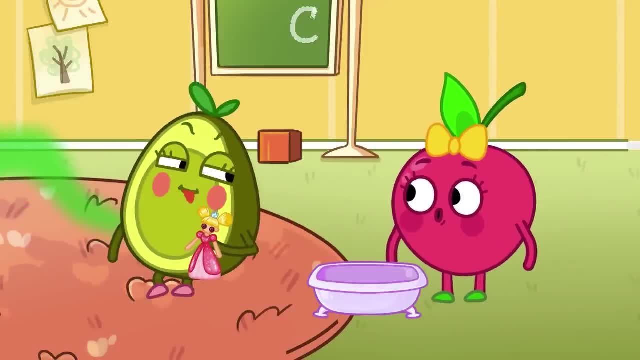 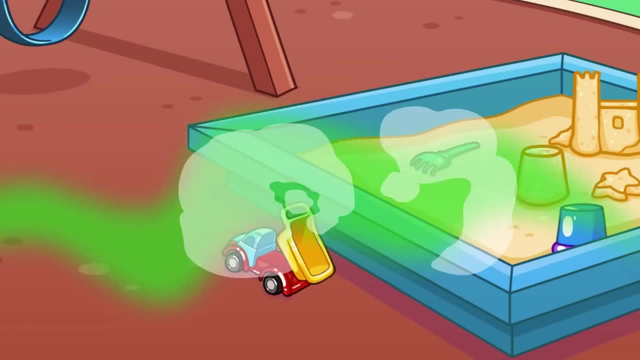 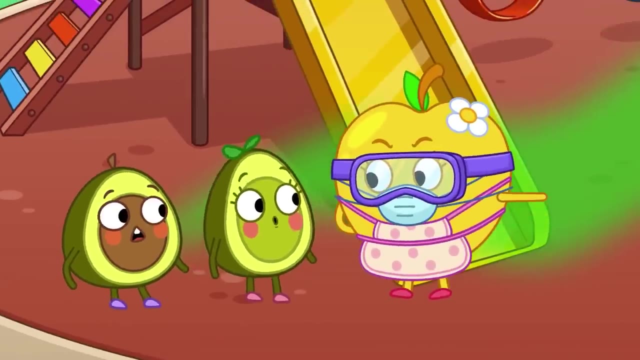 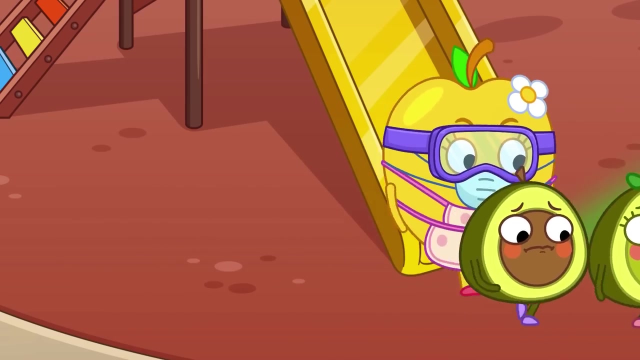 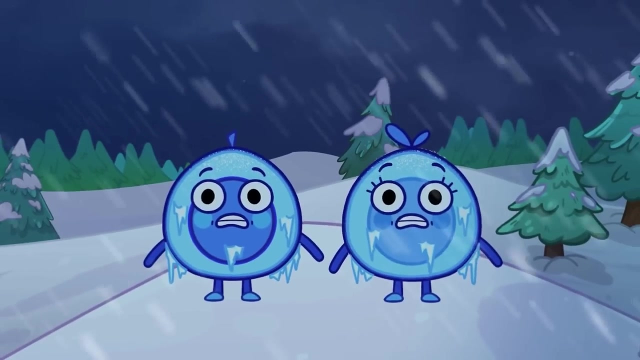 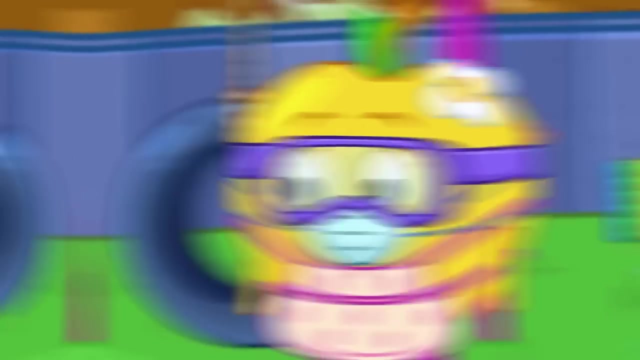 But Penny doesn't want to share with Lime. Penny doesn't want you. No one wants to play with Pit and Penny. Miss Apple sends them to wash in the pool. What's wrong now? This water is too cold. See how dirty you both are. 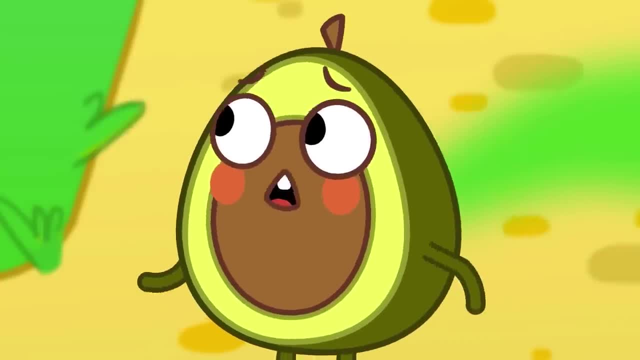 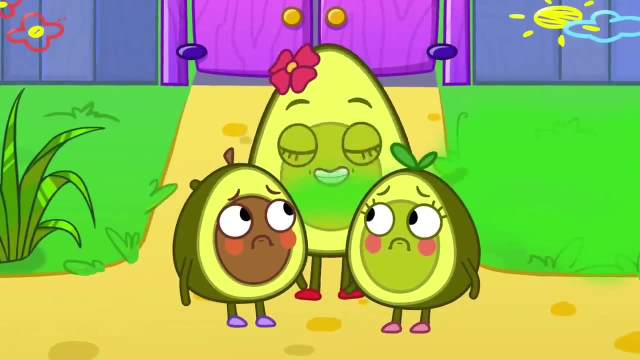 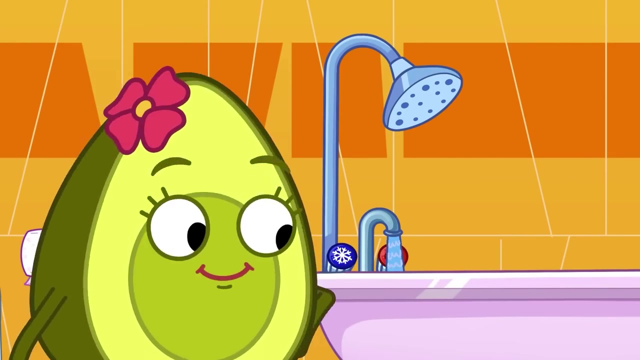 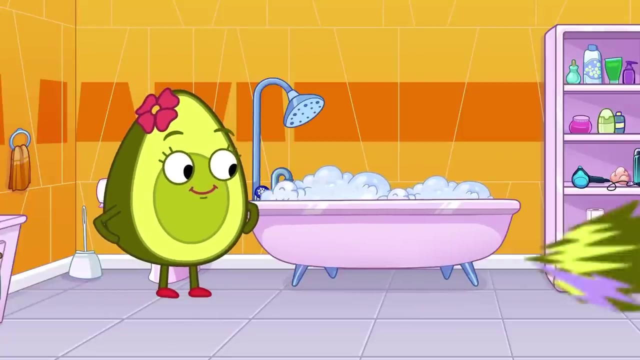 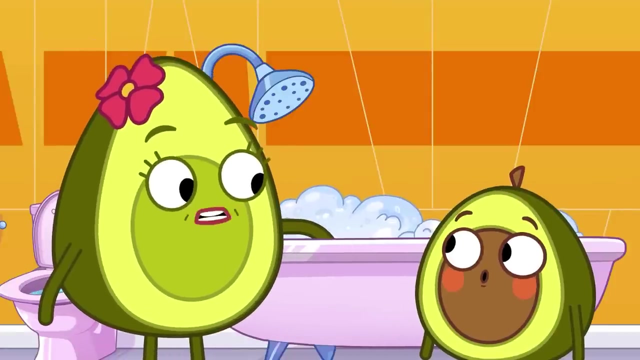 It's time to talk to Mommy. Mom, We need to bathe. Mommy adds bubbles to the bath. Don't forget little Ducky. It's ready, Ready. The bath looks amazing. The water isn't hot. See, It's perfect. 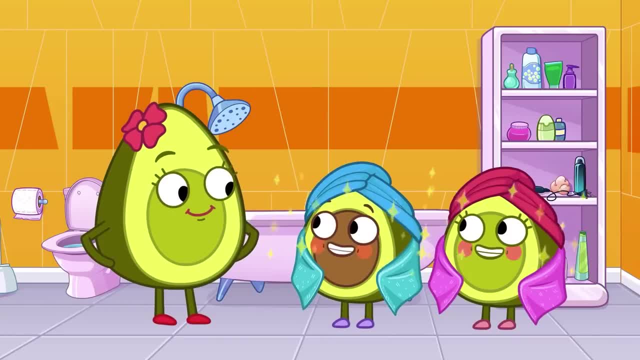 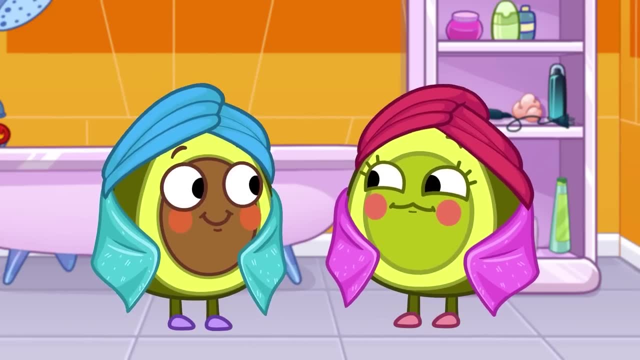 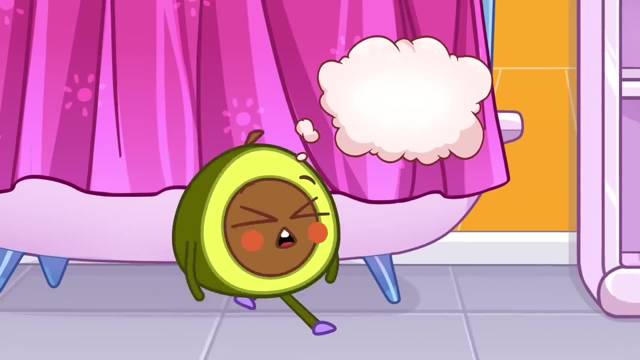 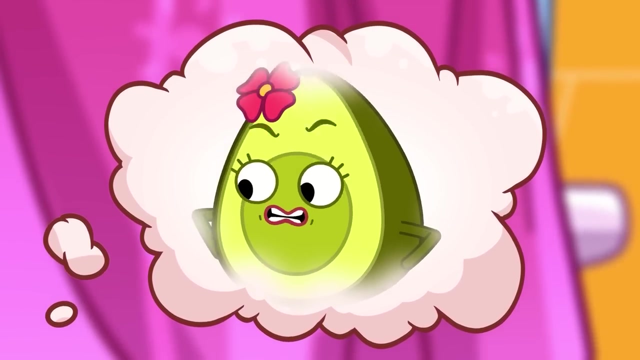 In you go Now. we'll never be afraid of taking a bath. Good job, Wait Pit. aren't you forgetting something? Pit, you need to wash up the toilet and wash your hands. What should Pit do now? Oh Pit. 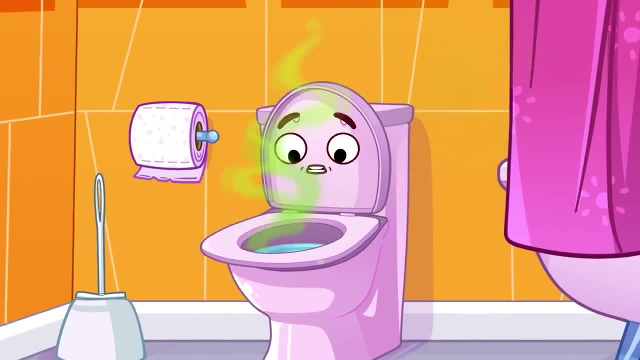 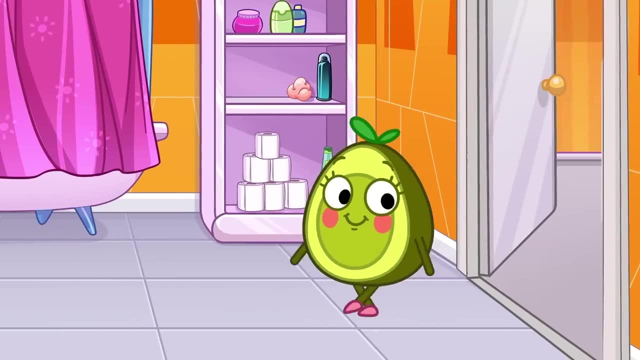 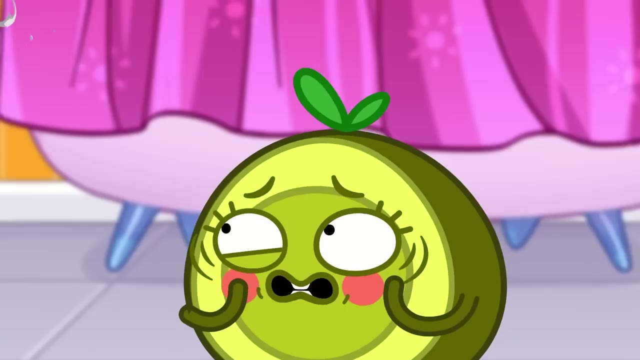 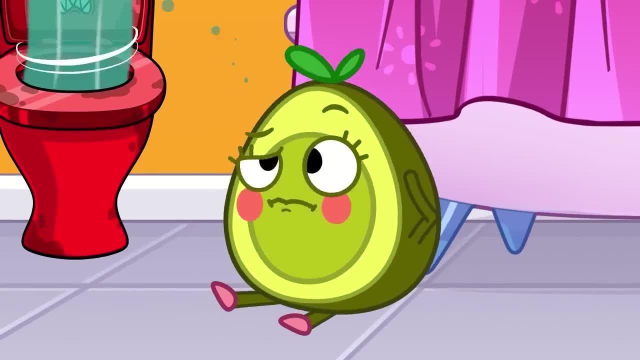 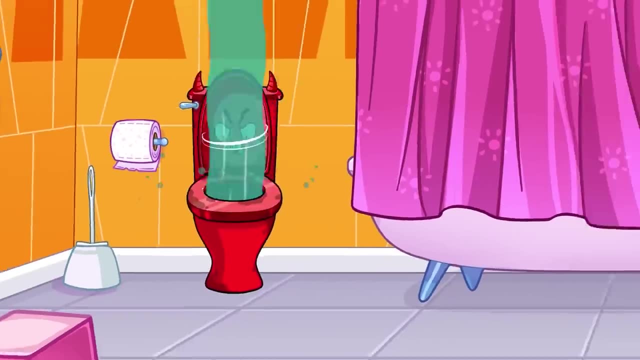 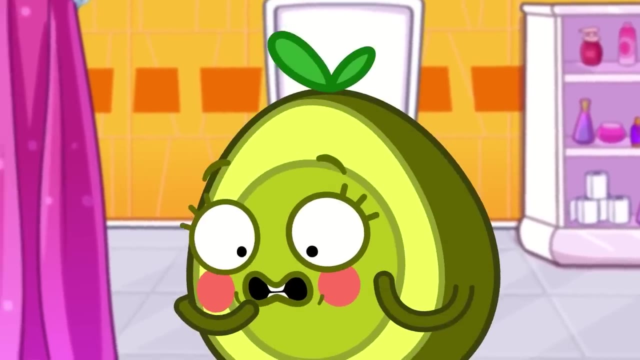 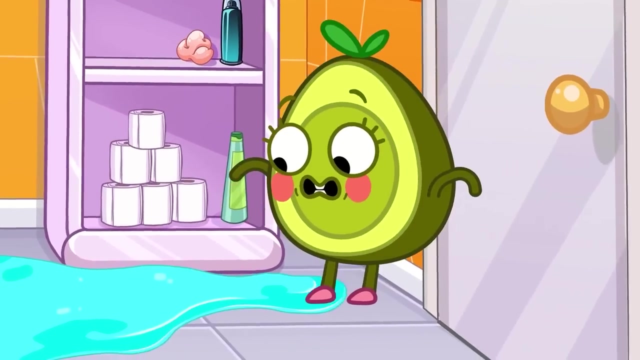 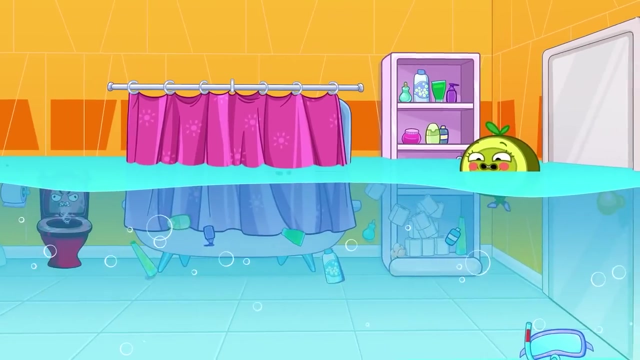 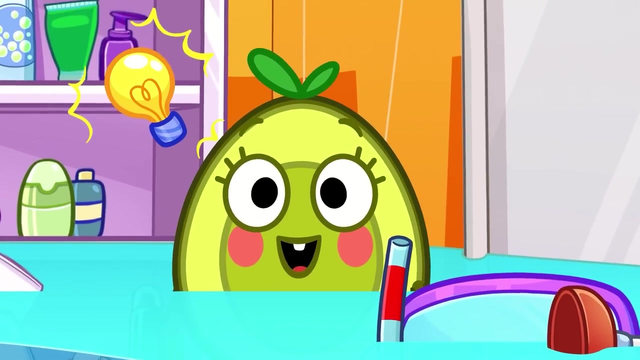 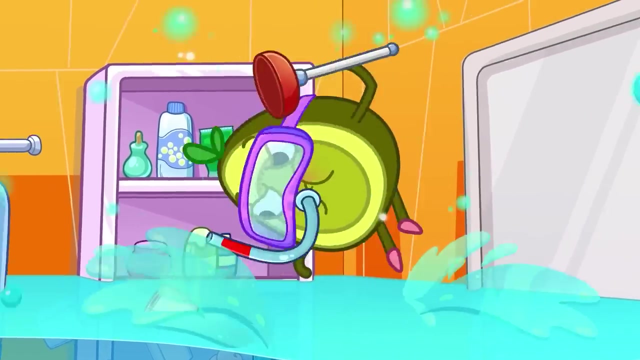 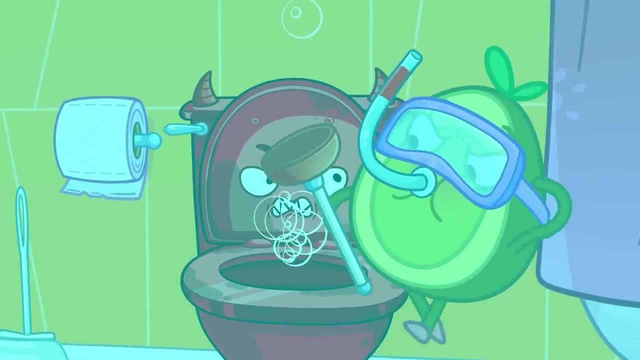 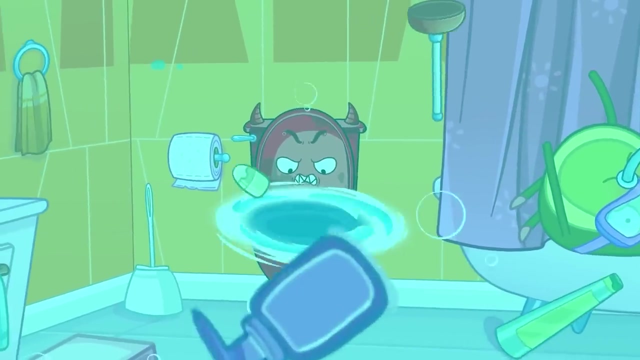 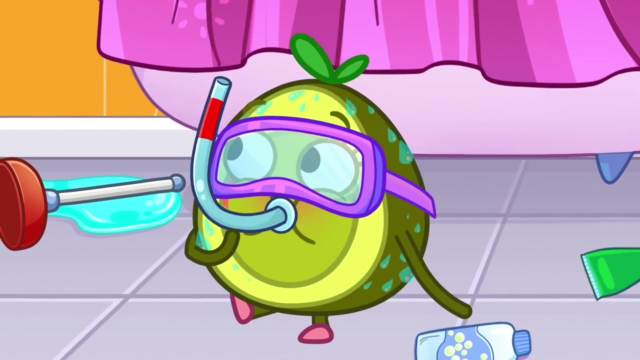 Don't get too close. Don't get too close. Poor Penny, Are you alright? The toilet is overflowing. Maybe that swim mask and plunger will help. Go get him, Penny. It worked, But the bathroom is a mess And the toilet isn't fixed yet. 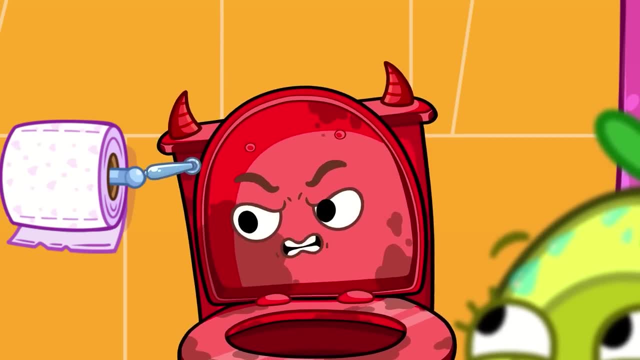 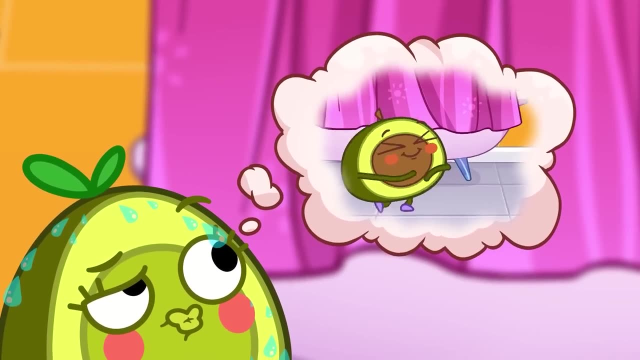 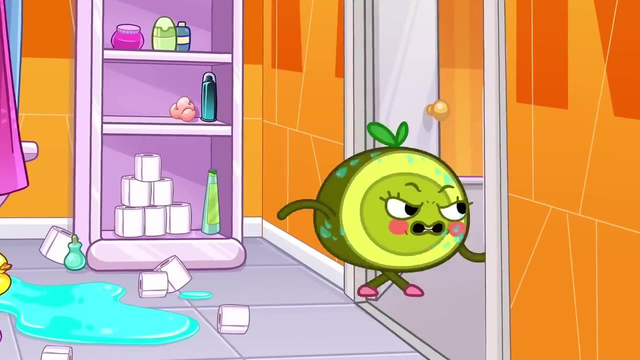 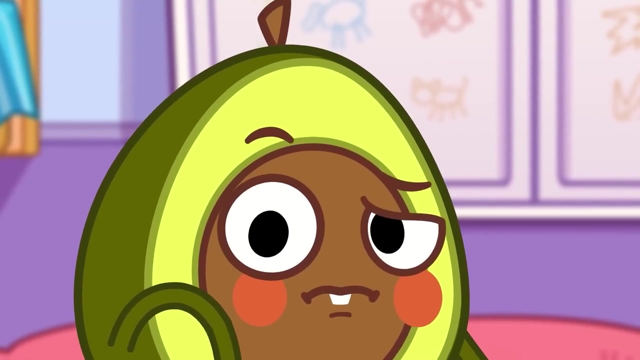 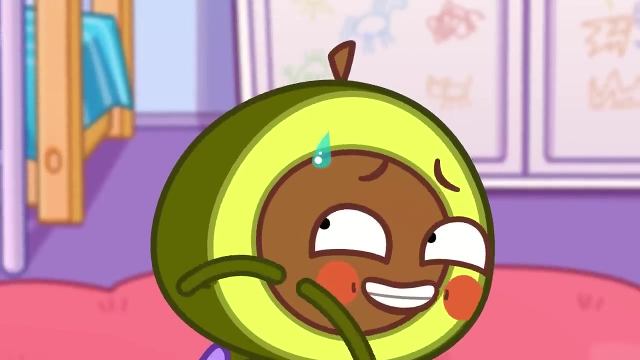 What's wrong, Mr Toilet? Whenever people don't wash me up, I get very angry. Maybe it's time to have a talk with Pit. What's dripping on your head, Pit? It's a very unhappy Penny. Ah, Ah. 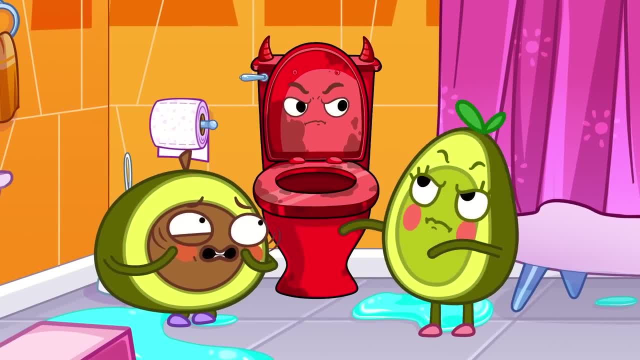 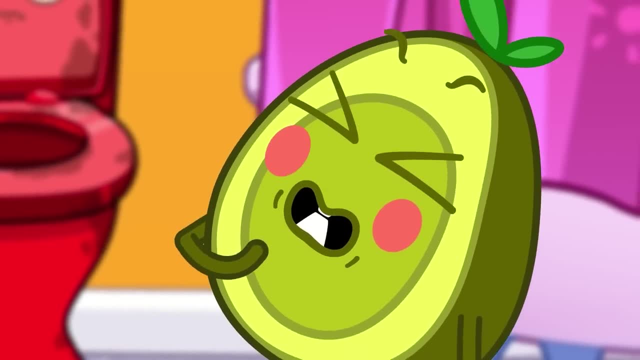 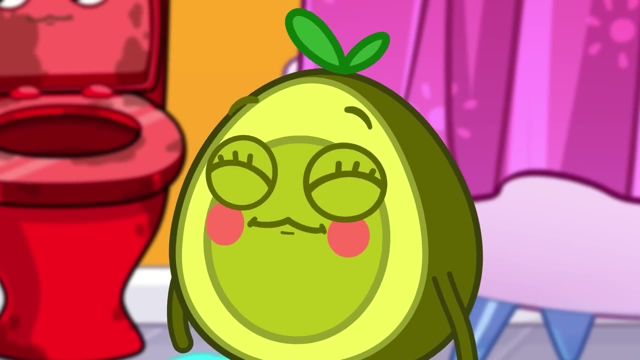 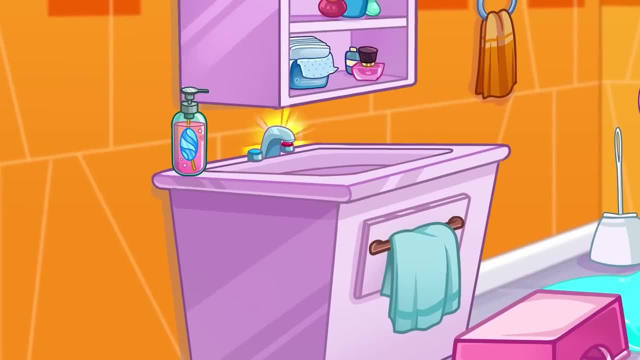 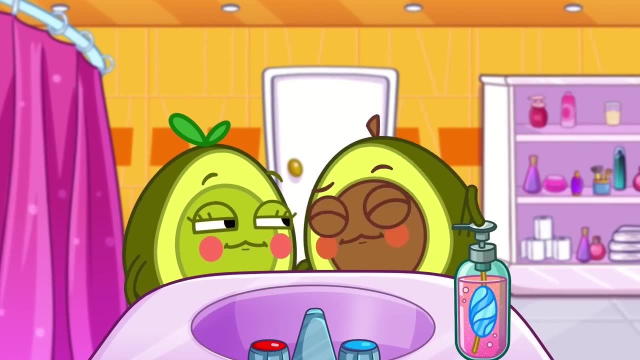 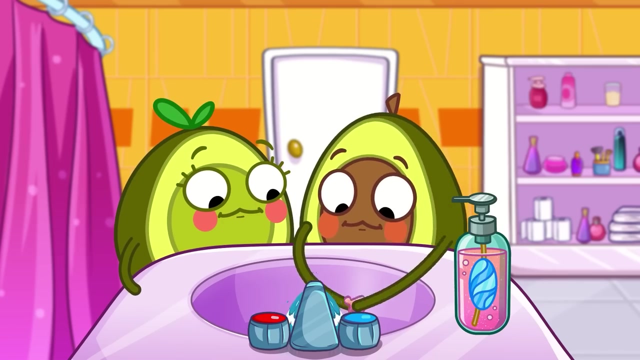 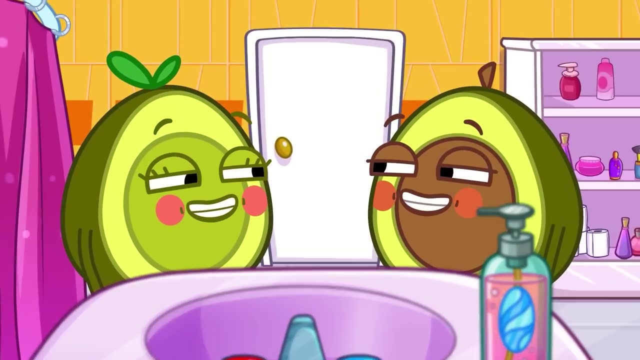 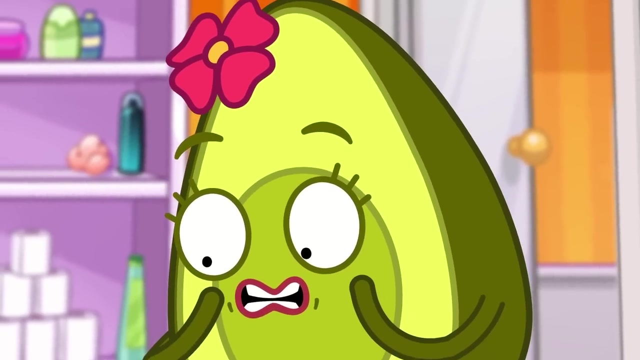 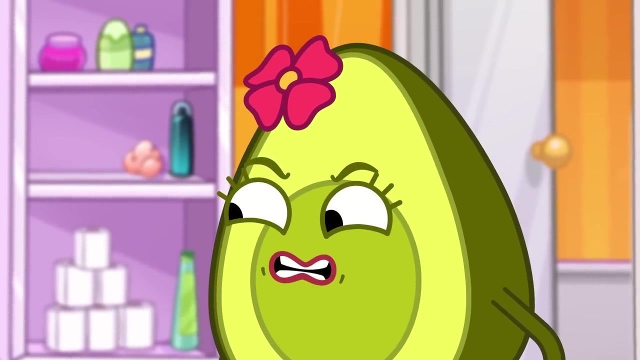 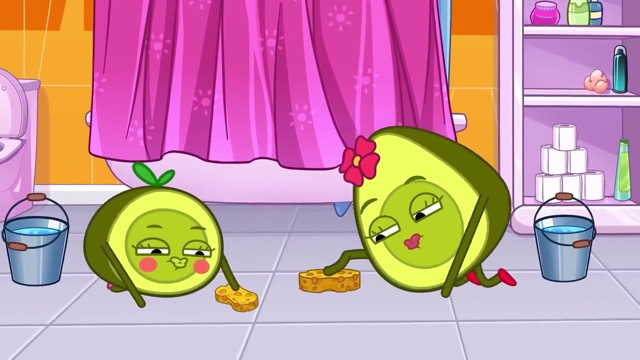 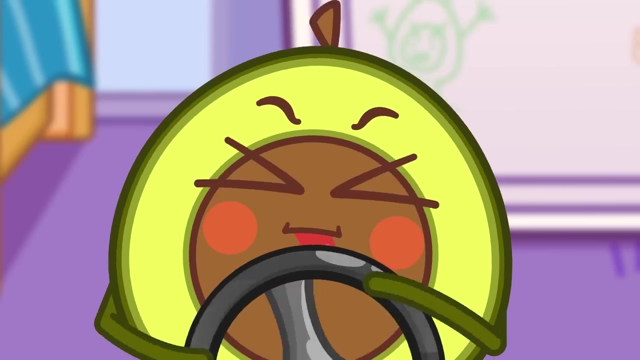 What else are you forgetting, Pit? And you should always wash your hands. Kids, you have to clean up here. The bathroom is looking nice and clean. Good job everyone. Pit is racing his black car And Penny is racing her pink one. 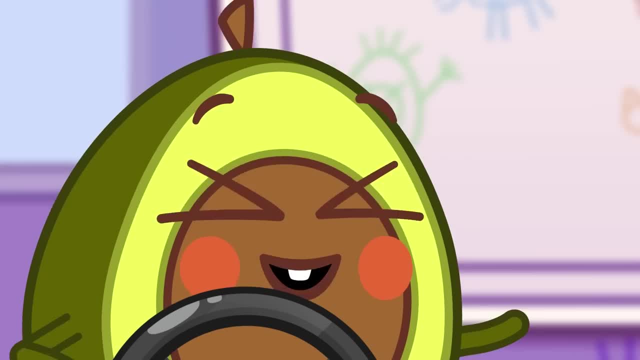 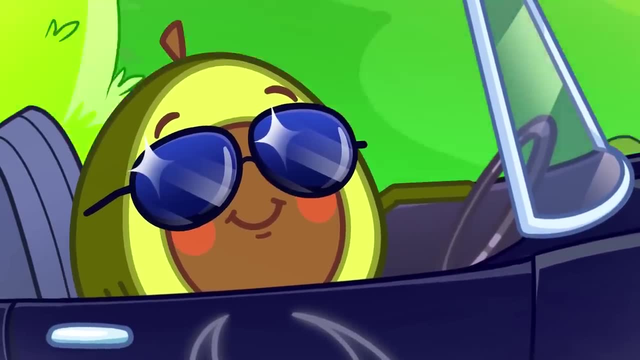 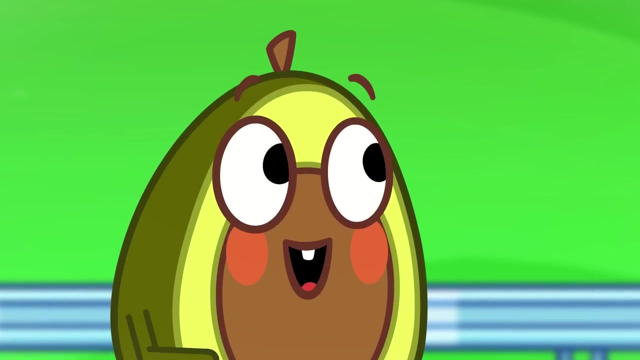 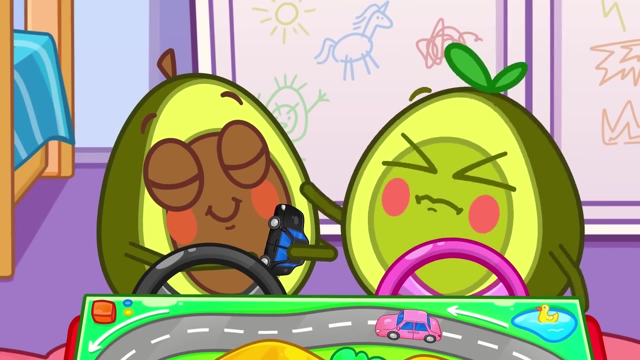 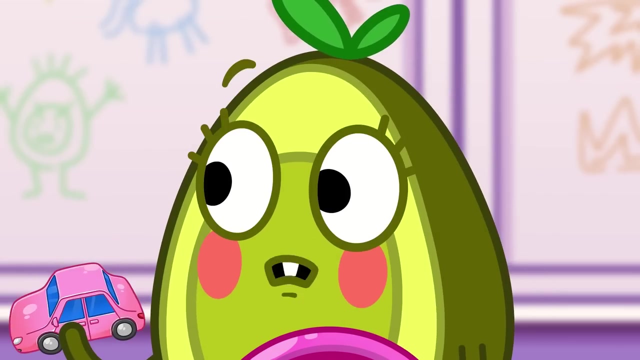 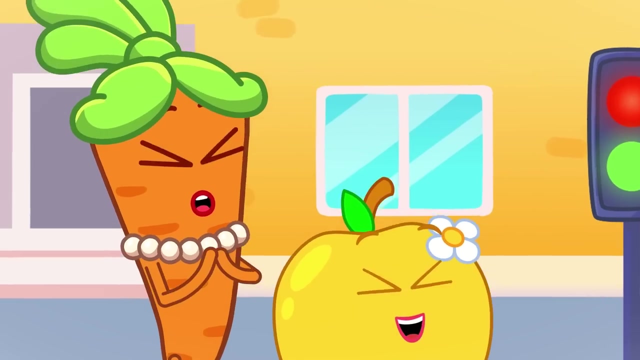 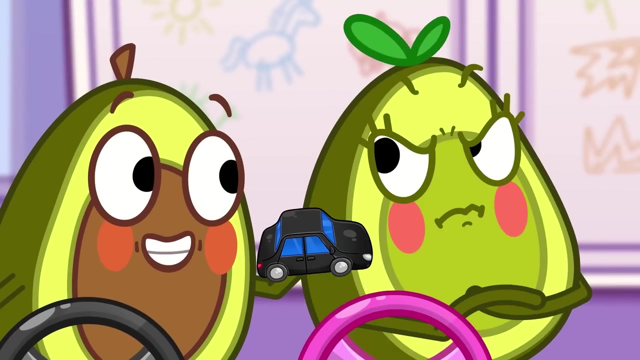 Who's going to win? The black car is better than pink. Pit looks very cool in his black car. What do you think, Penny? The pink car is the best. Penny looks very cool in her pink car. Is one car really better than the other? 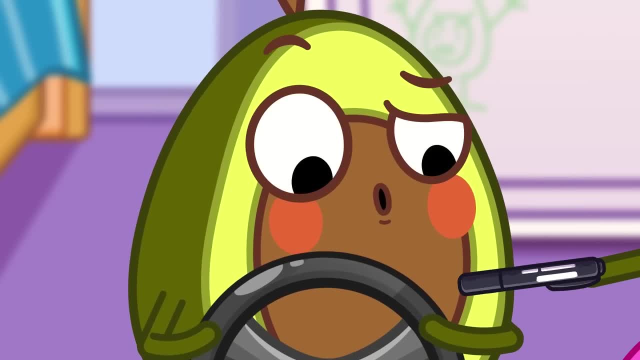 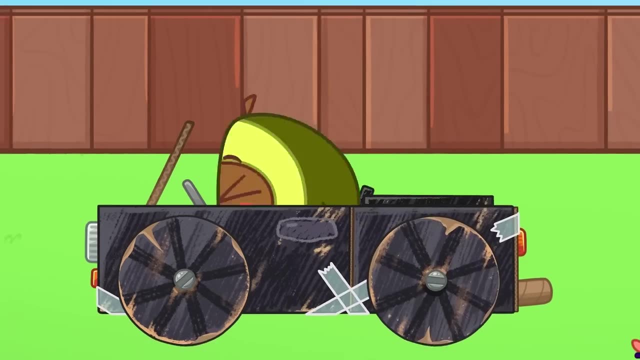 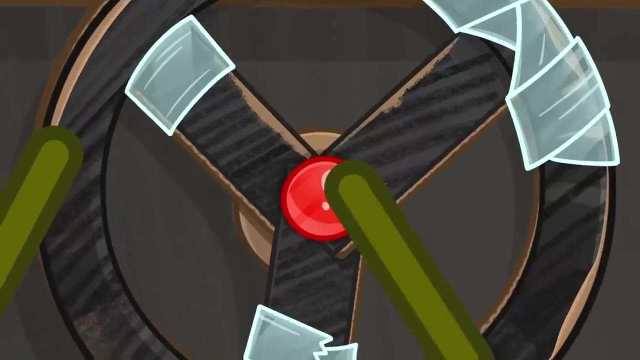 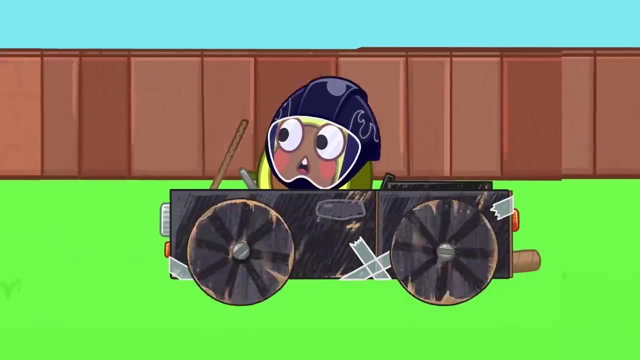 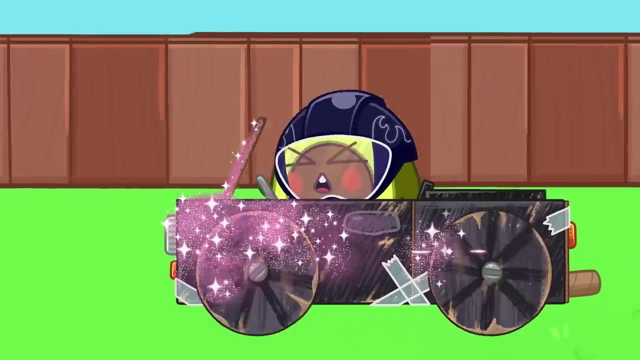 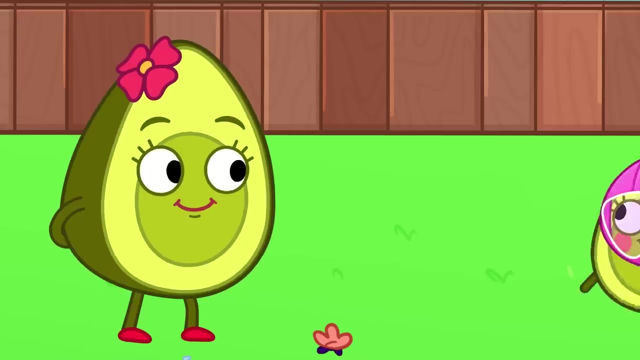 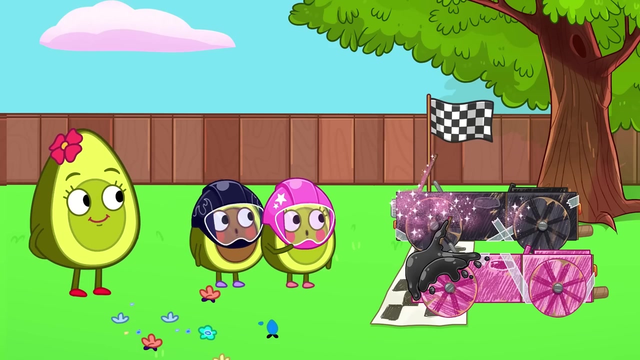 Penny has an idea. There's going to be a race. Watch out Penny, Watch out Pit. Here comes the finish line. Mommy will decide who won. You crossed the finish line together. Both our cars are good. It's a tie. 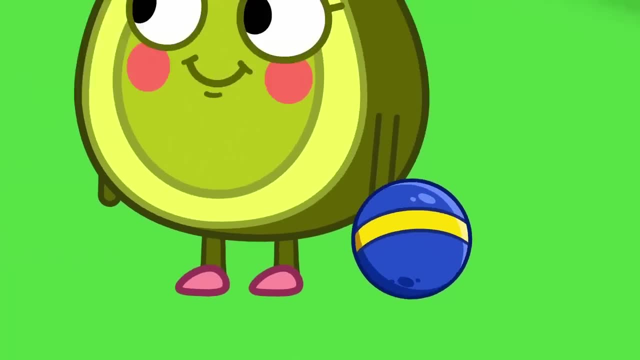 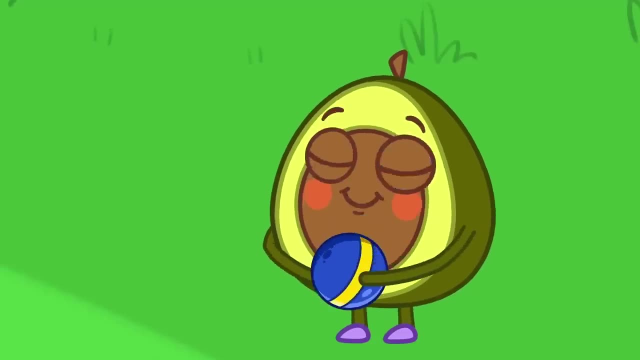 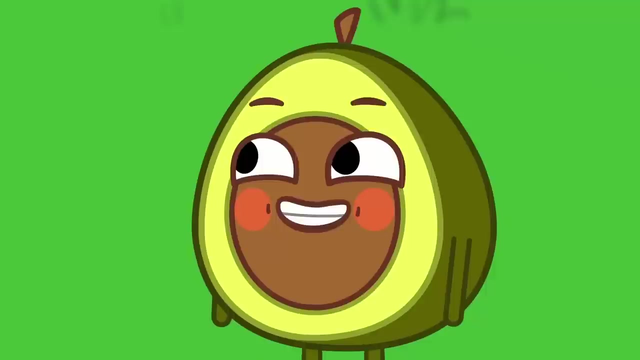 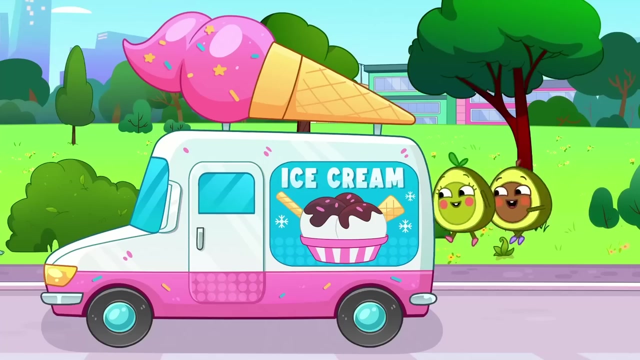 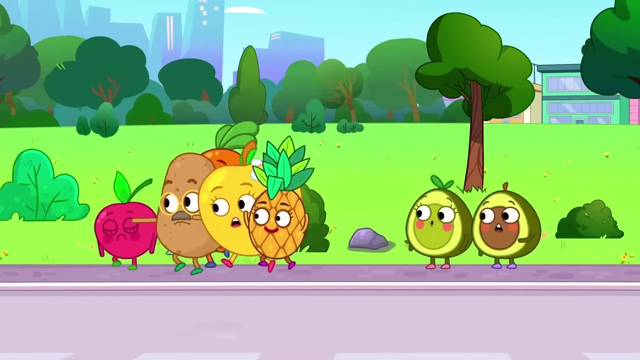 Enjoy your trophy. Pit and Penny are in the park. They're playing catch with Daddy. Everyone is having fun. Smile. What's that noise? Don't run far away. It's the ice cream truck. Yummy, I think everyone wants ice cream. 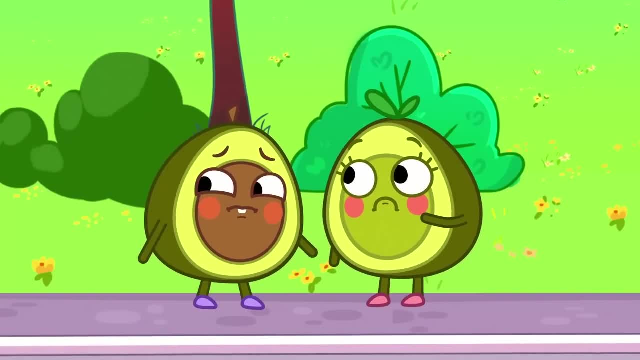 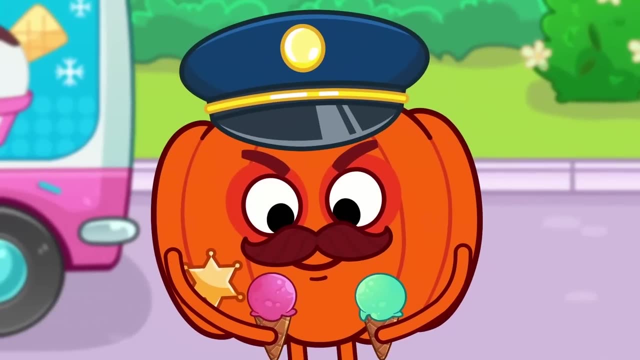 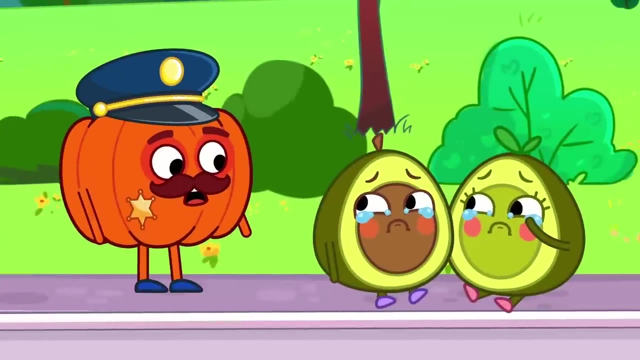 Come on, kids, just play with your daddy. Okay, Everybody get a little joyous. We've got everyone looking delicious. Do you like this ice cream truck? Give it Nuh-uh, Can you drive? Oh, Mommy. 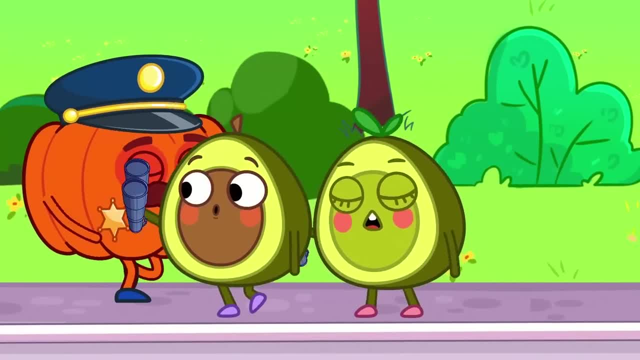 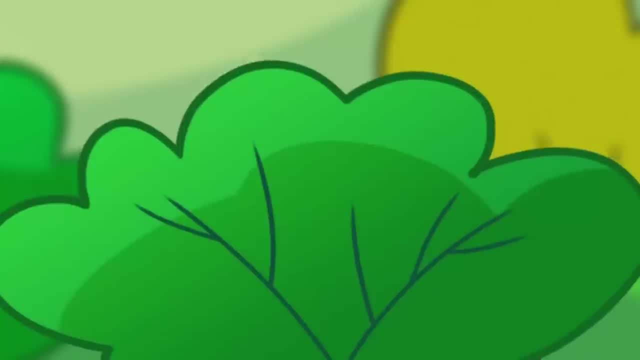 I have a kayumbi. yeah, I was going to stop by. I was hoping I could find something. We've got 600!. Mom and Dad, Pete and Penny, are looking for you. Mommy and Daddy are worried. That's not Pete and Penny. 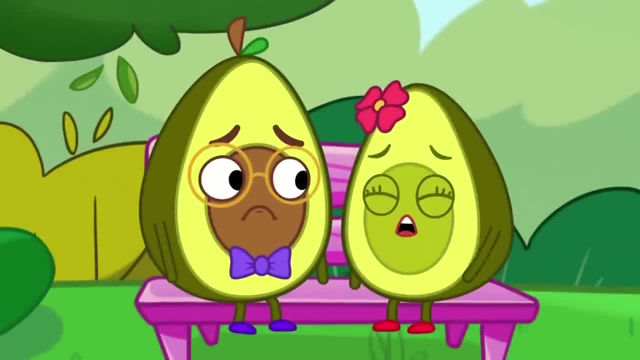 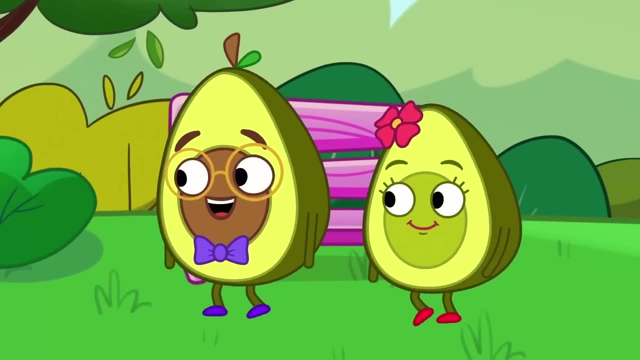 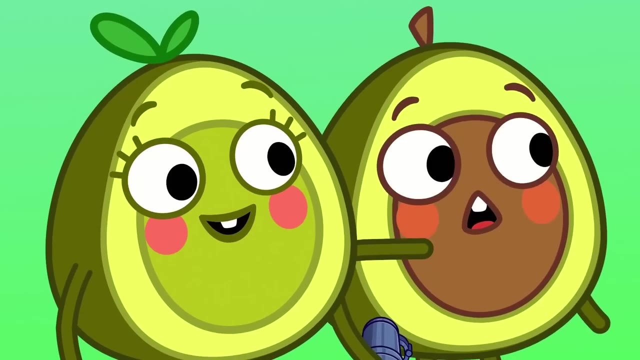 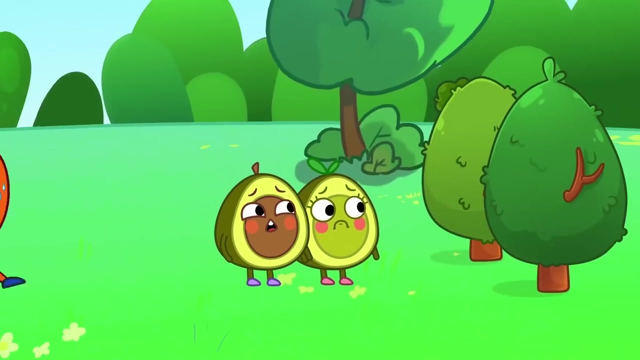 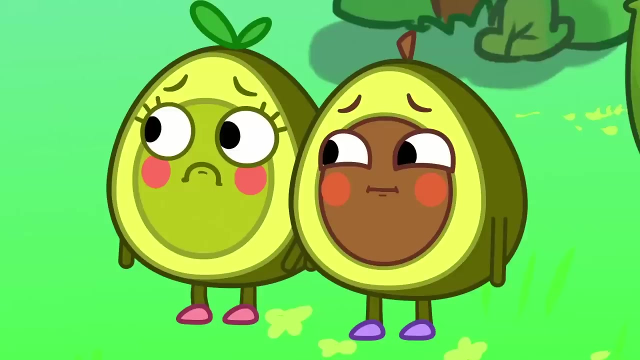 That's a squirrel. Children, where are you, Mom and Dad? where are you? Can you see Mommy and Daddy? Where are you? Hmm, that's not right. These are not your parents. These are bushes. Pete looks for Mommy and Daddy. 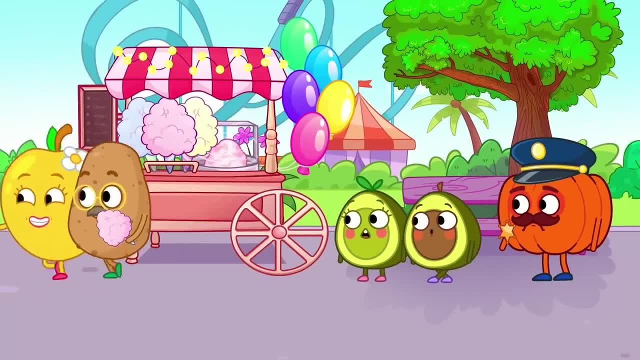 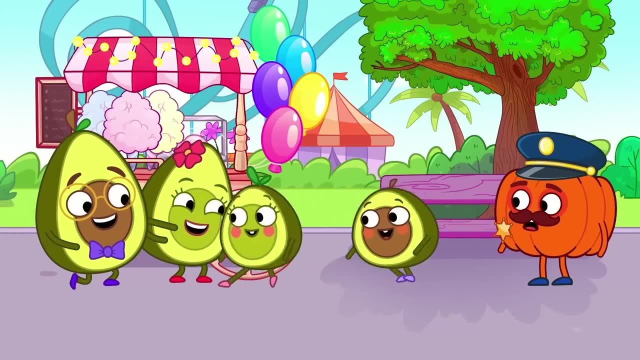 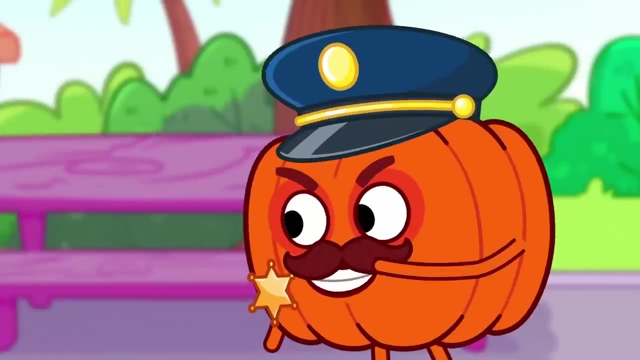 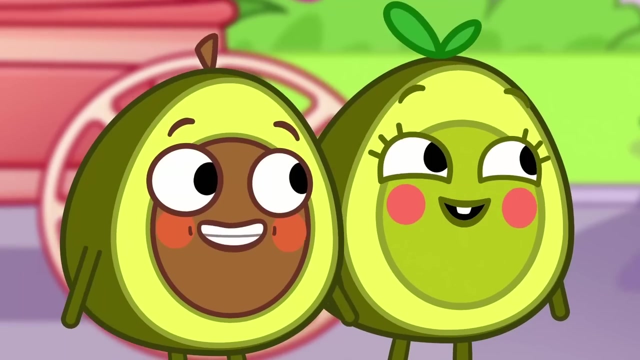 Look over, there Are these your parents. It's me, Mommy and Daddy. Officer, thank you very much for finding our children In public places. do not leave your parents. Stay close to them. Thank you very much. This is for you. 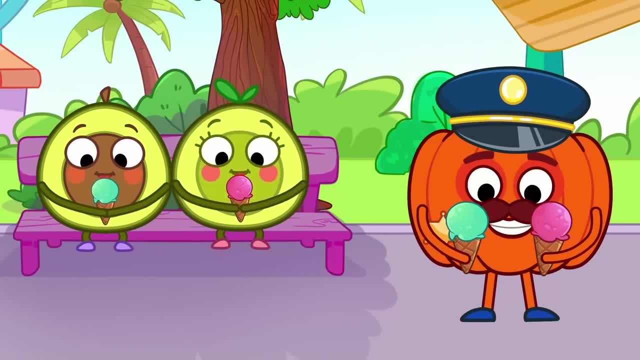 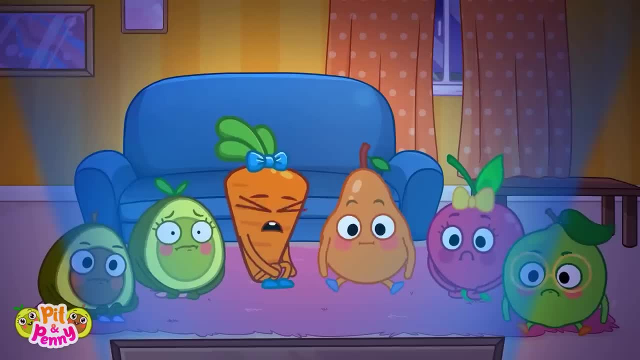 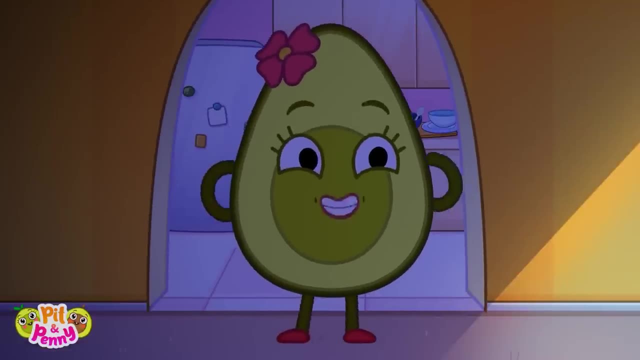 Officer Pumpkin loves ice cream. The kids are watching a scary scene. It's like a zombie movie. Who's that in the shadows? It's time to go to sleep, kids. It's only Mommy Phew, Okay, Okay. 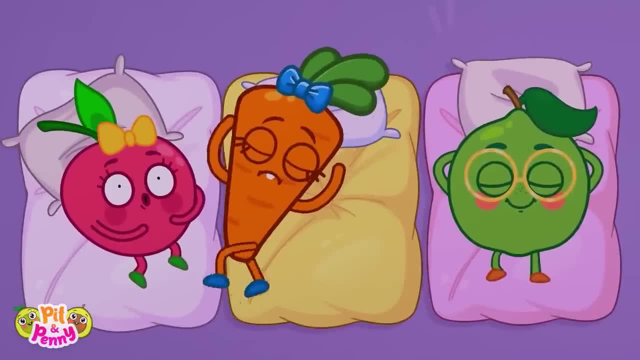 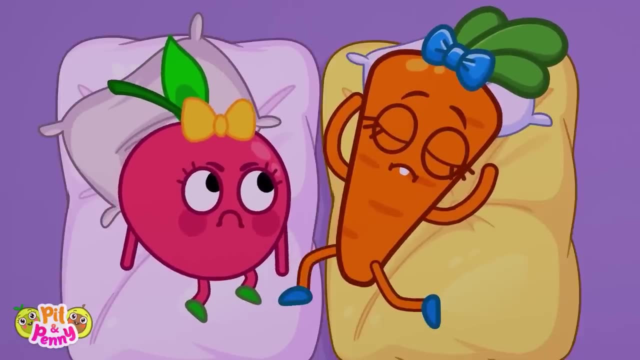 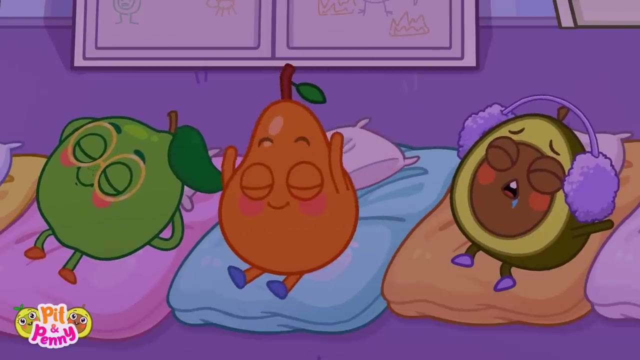 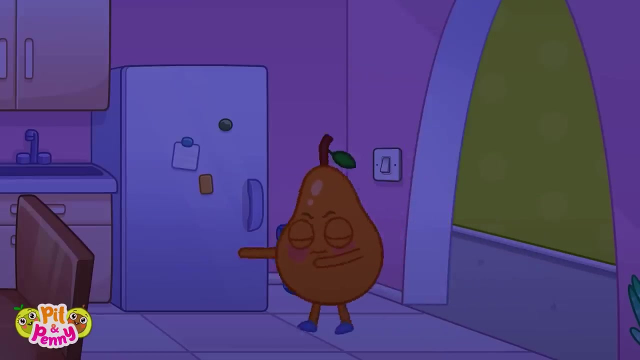 Carrot is having a bad dream. Carrot is having a bad dream. She's woken up Cherry. What's going on? Help, Cherry might have to sleep somewhere else. Hair is sleepwalking. Where is he off to Help? 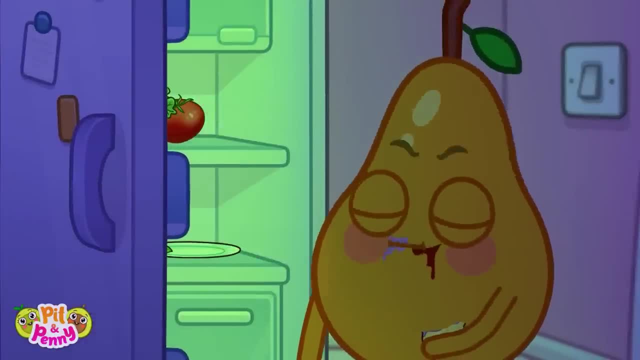 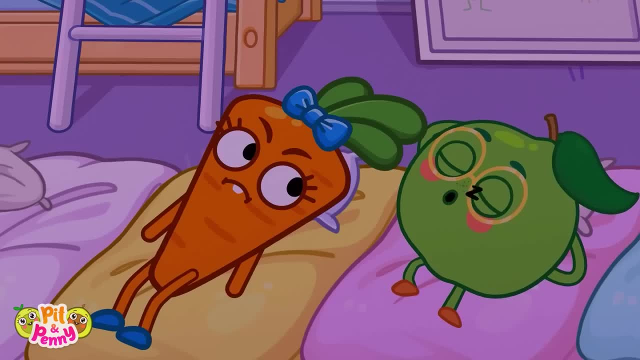 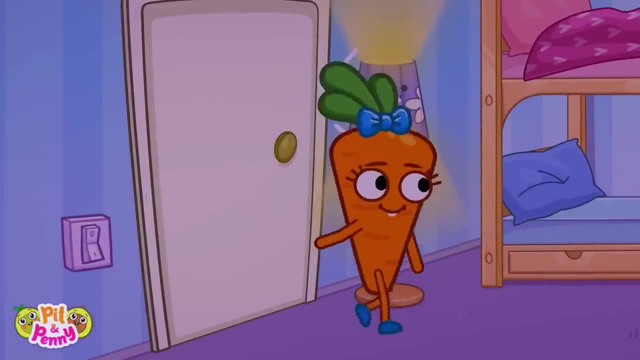 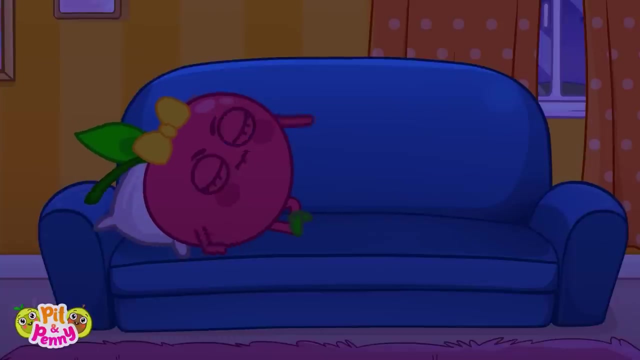 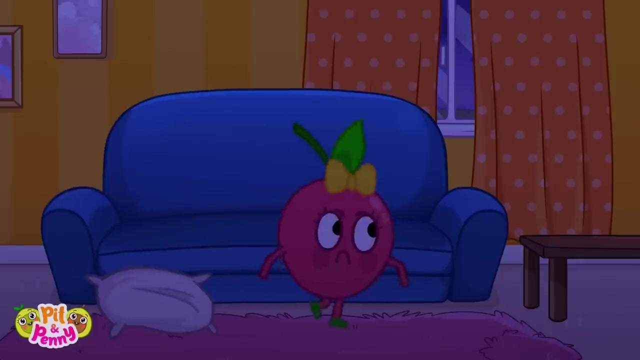 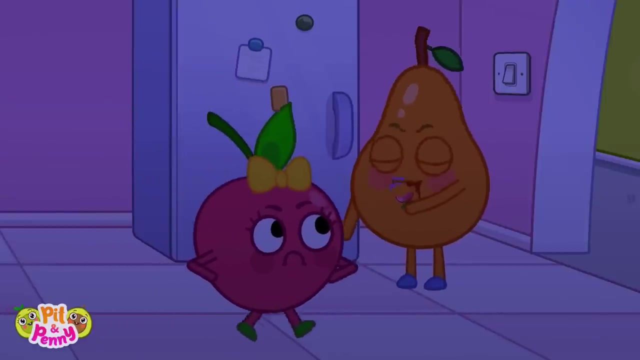 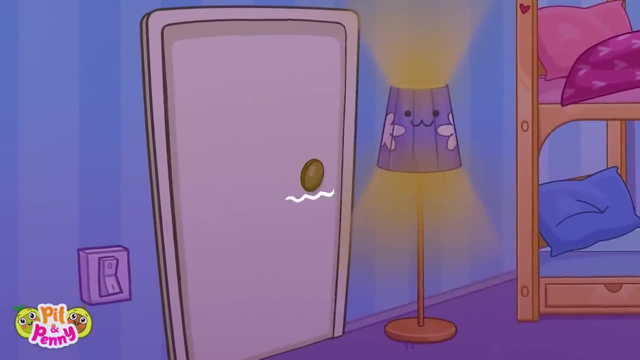 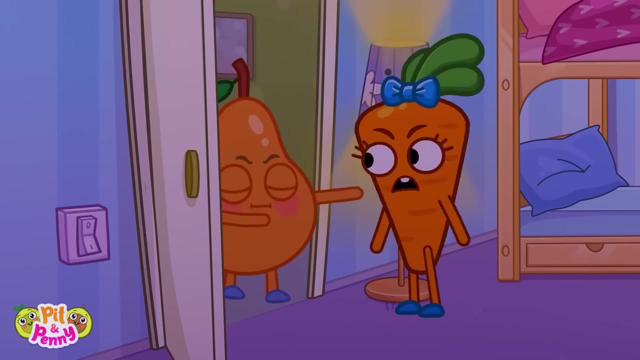 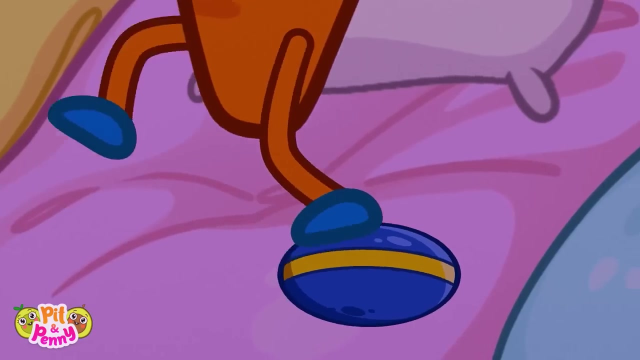 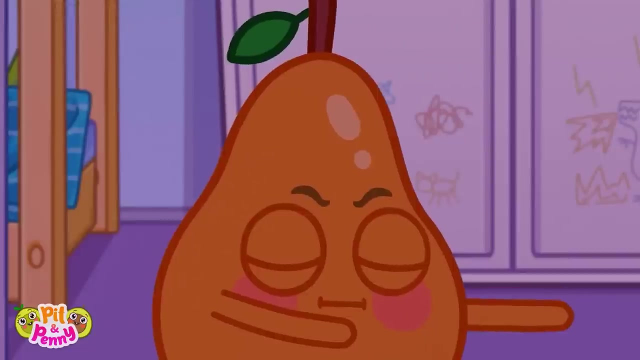 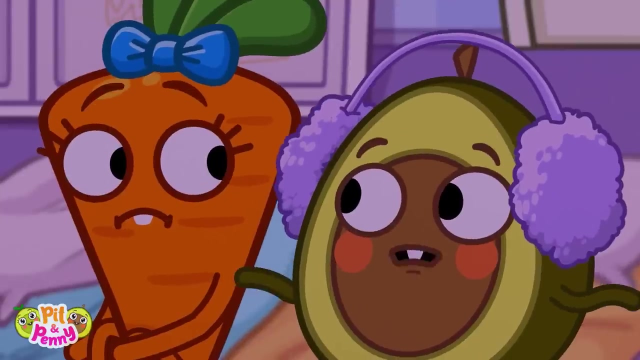 Shh Pit and Penny are still asleep. Maybe now Carrot can get some sleep. Pair's eating is keeping Cherry up. That's better. Who's at the door? Carrot thinks Pair is a zombie. Watch out What. Nobody's sleeping here. 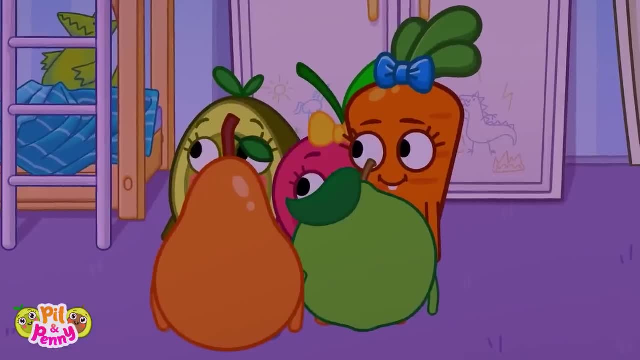 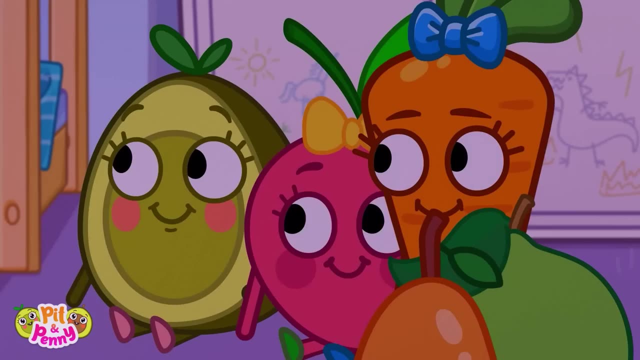 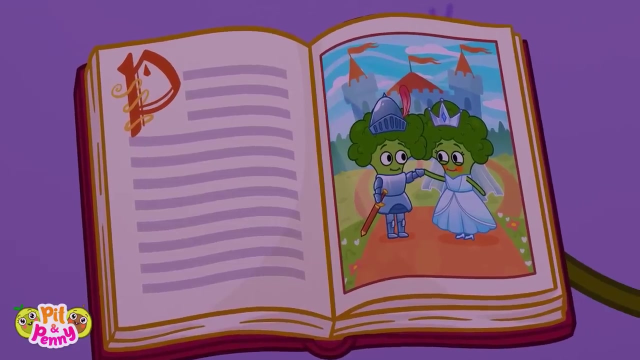 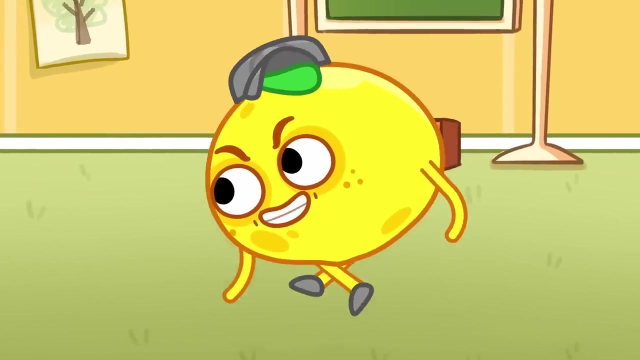 What is your idea, Pit? Let's read a fairy tale. A few minutes later, Happily ever after The end, It looks like Pit's bedtime story worked. Night kids, Sweet dreams. Be careful, Little Lemon, Oh no. 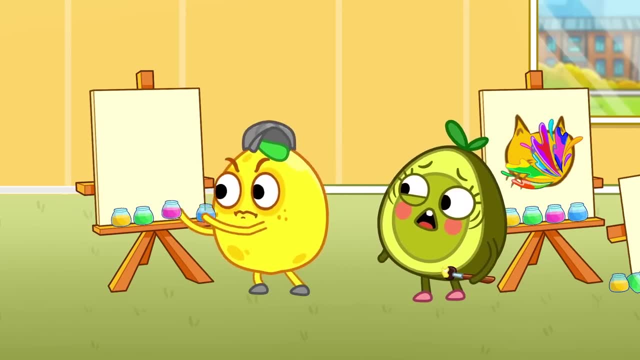 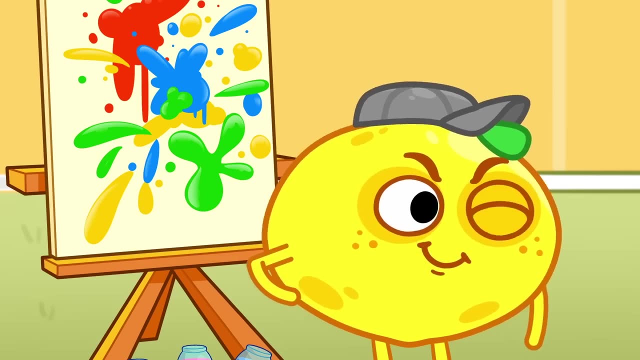 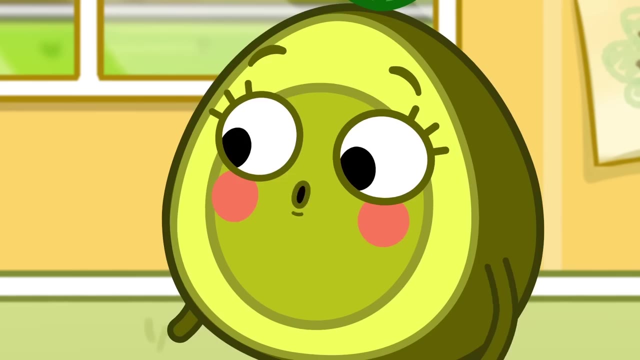 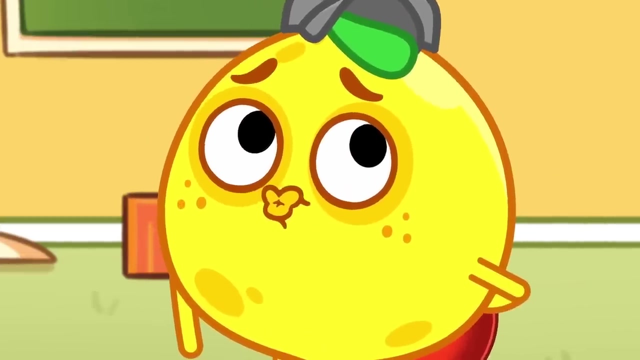 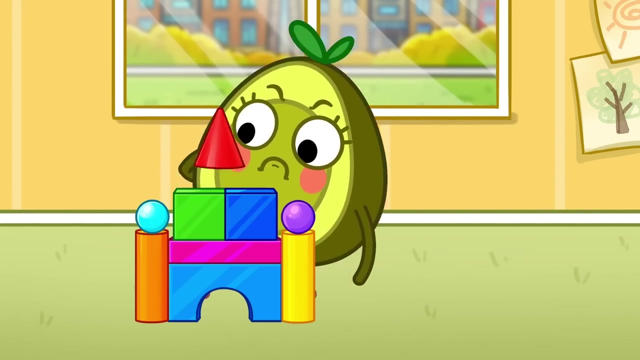 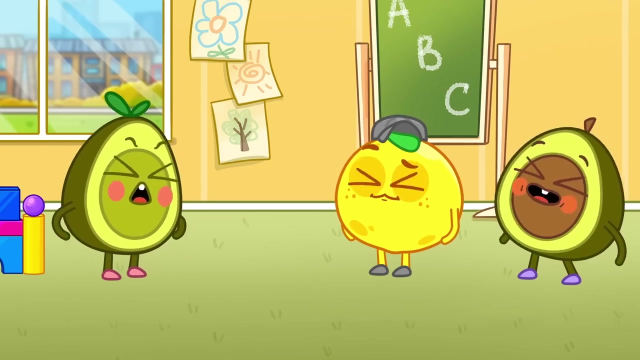 Look at the mess he's making. It isn't very funny, Pit, Well done. Who did that? Okay, I know, it was you. Oh, the boys did it again. Stop it, boys, Don't do it, Bid. 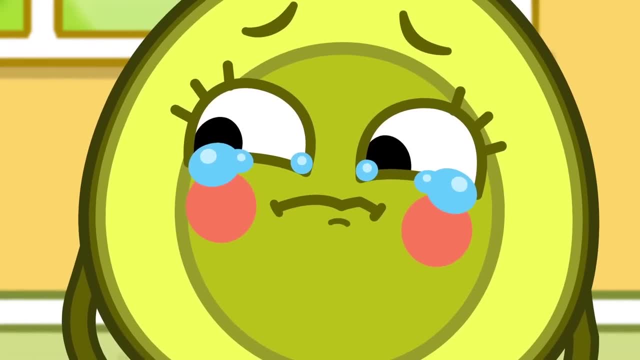 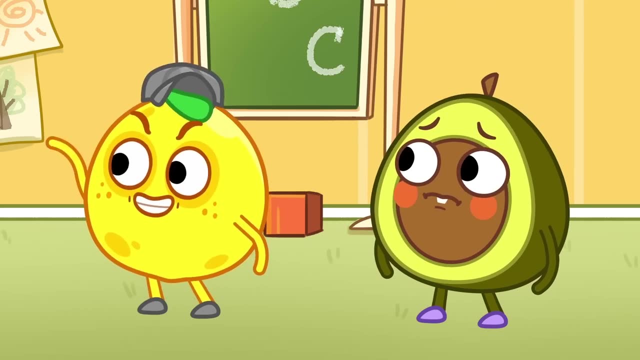 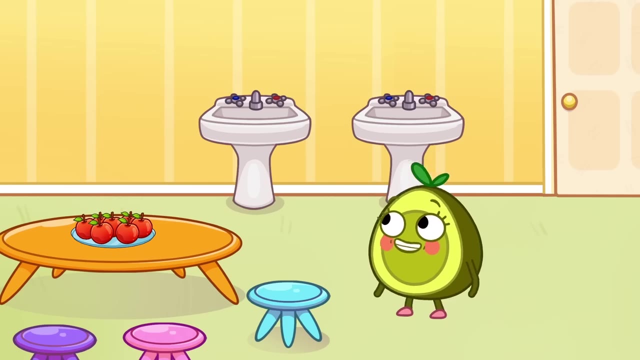 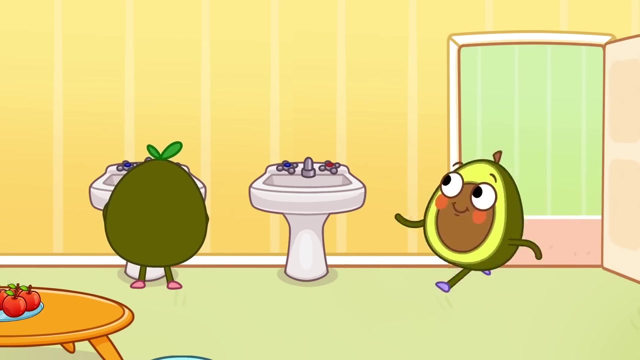 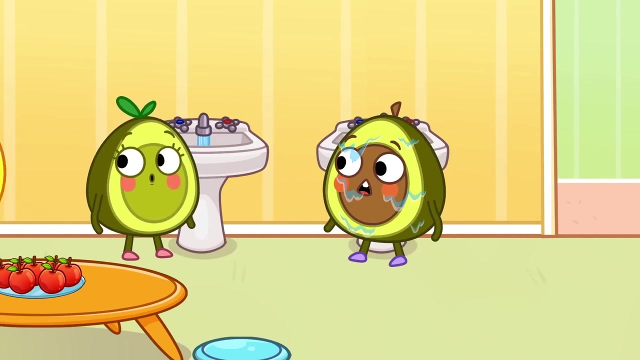 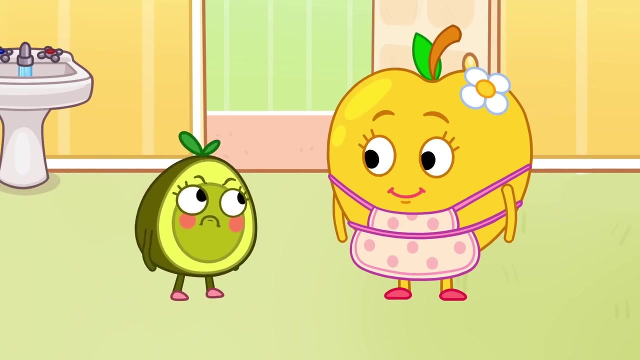 And his castle is ruined. This is bad behavior, Bid. Look some yummy apples. First I need to wash my hands. What a good idea, Penny. That's not nice little lemon? That's it. It's okay to ask a grown-up for help. 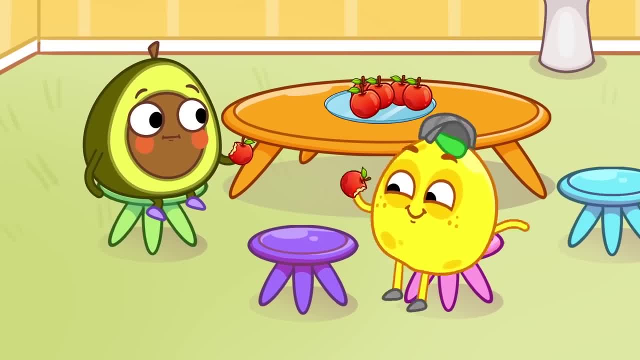 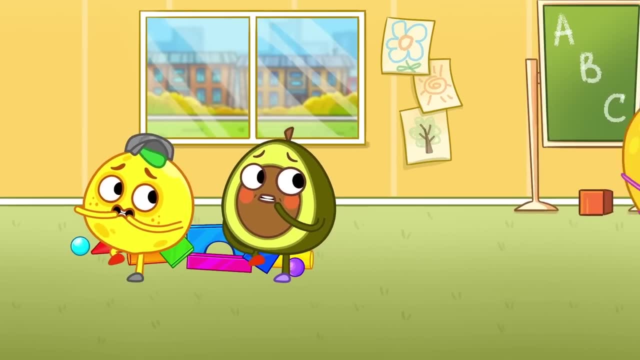 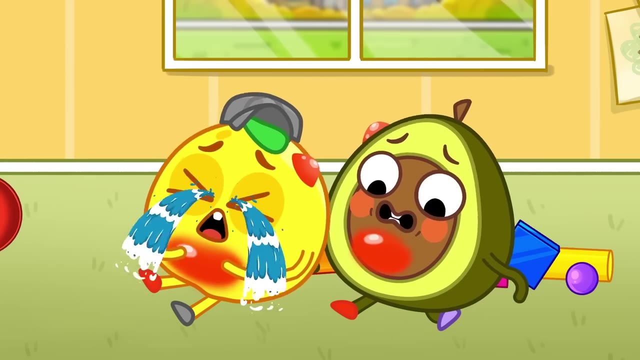 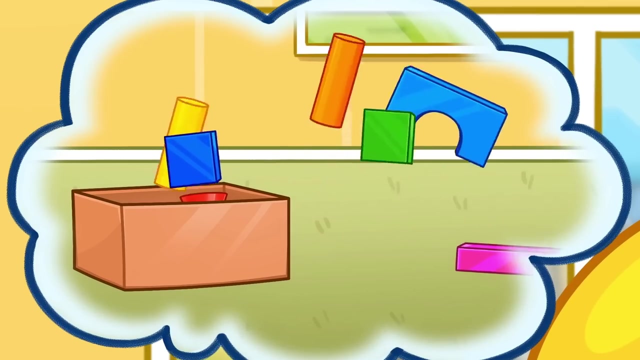 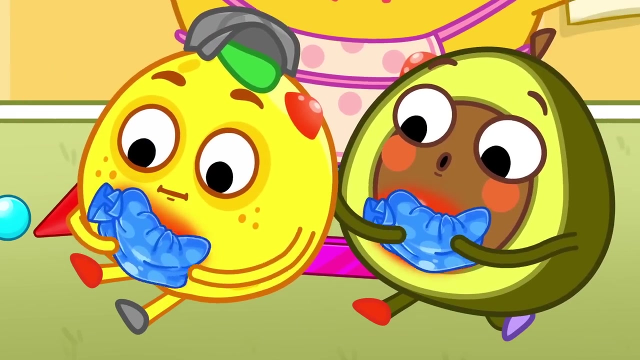 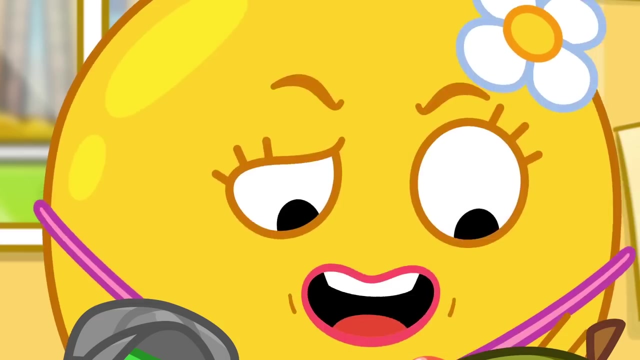 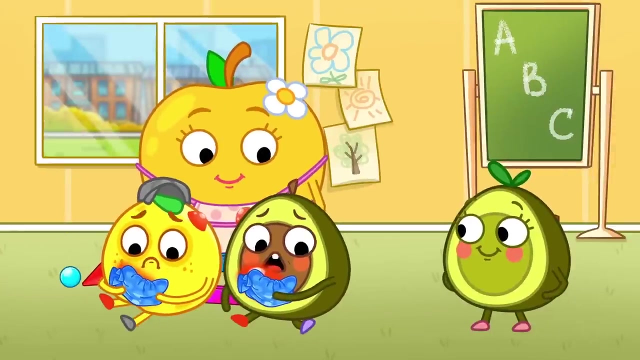 When being bullied or teased. Bad things happen when you misbehave. Miss Apple will help. Just remember: Don't throw your toys around. Wash your hands before you eat To get rid of germs that make you sick. We are sorry, Penny. 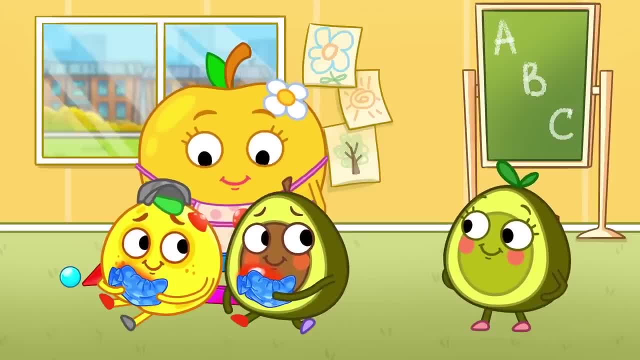 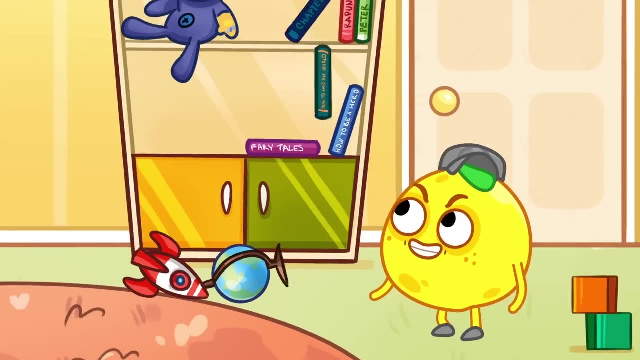 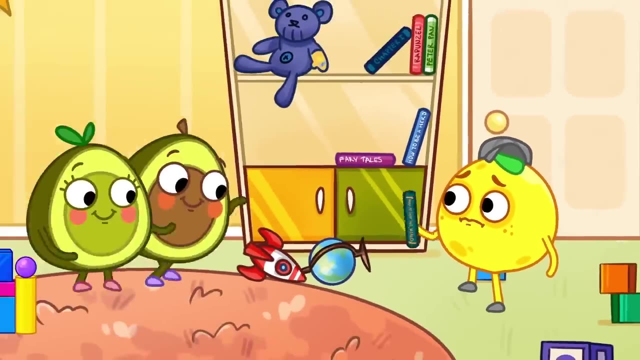 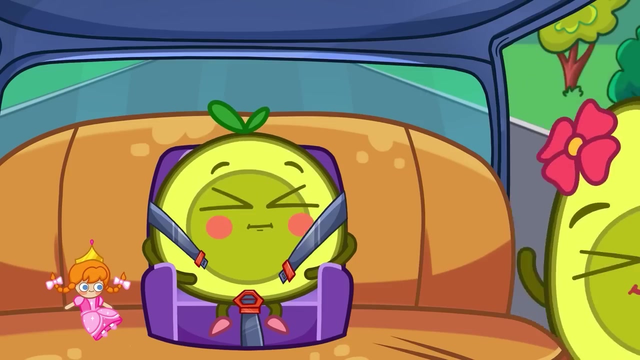 Be good and everything will be fine. Nice job. Little lemon is still not behaving. Oh sorry, That's much better, little lemon. Penny is going for a car ride. Mommy helps her buckle up the seatbelt. What? 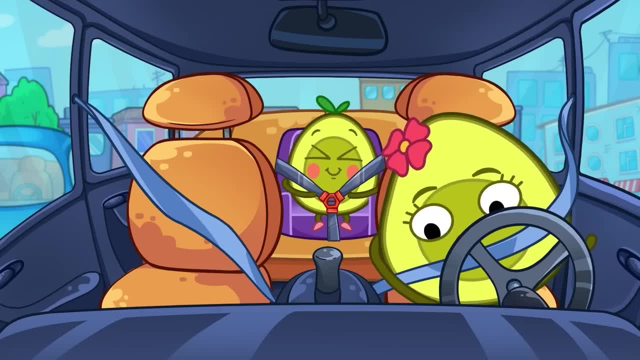 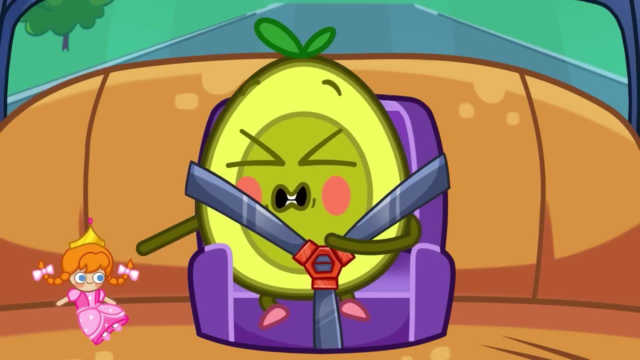 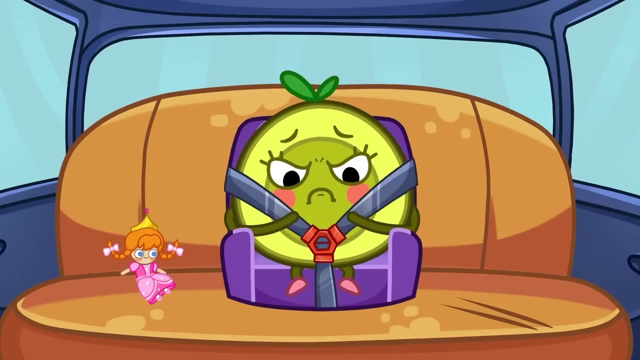 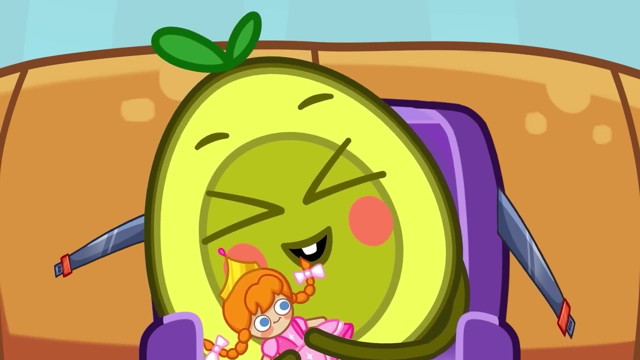 Don't forget your seatbelt. Mommy Penny wants her doll, but she can't reach it. Her seatbelt is in the way. Penny, don't unbuckle your seatbelt. That cat is sitting in the middle of the road. 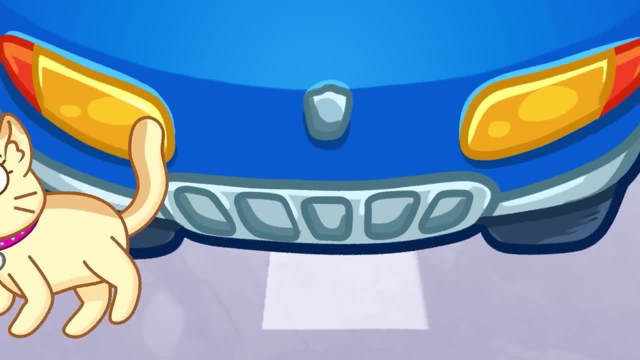 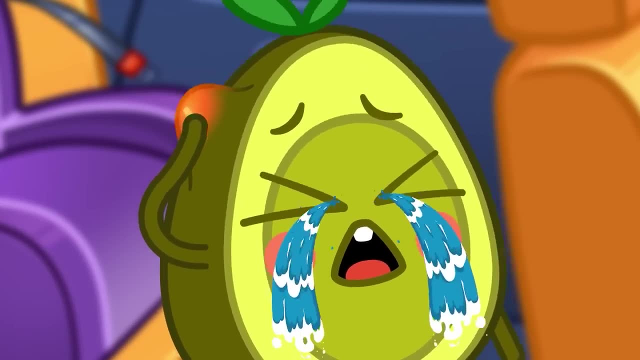 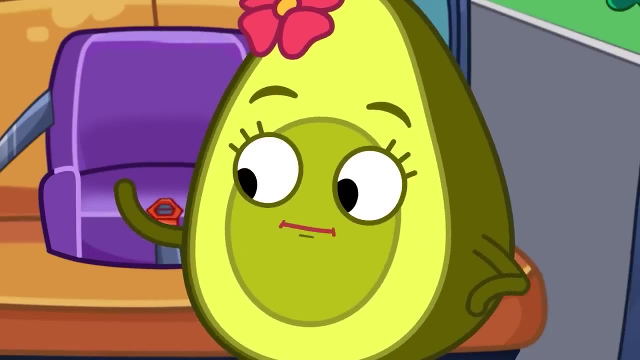 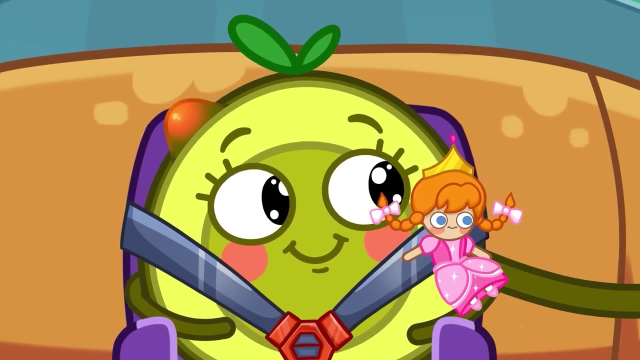 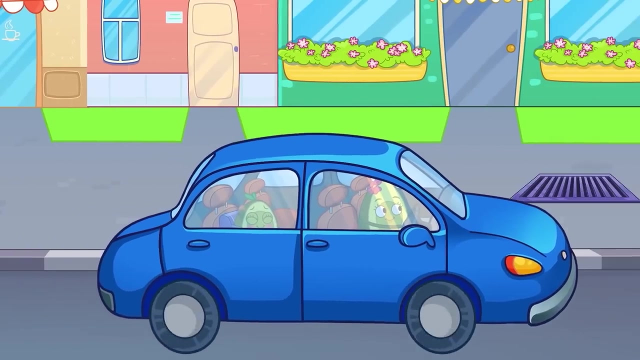 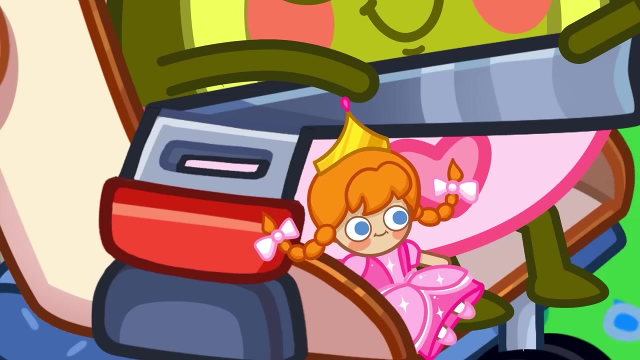 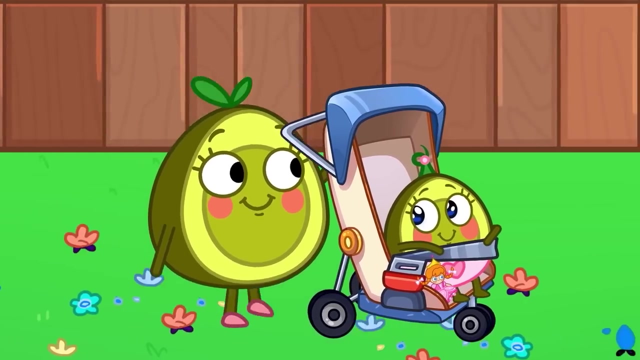 Phew, The cat is safe, But Penny bumped her head. You should always buckle up your seatbelt. Seatbelts keep us safe. Penny is playing with Baby. She makes sure Baby puts on a seatbelt. Oh no, A rock. 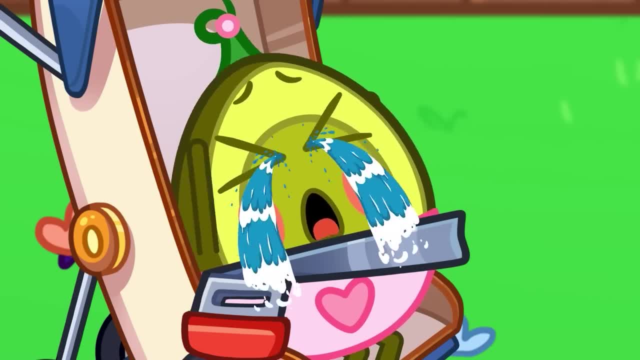 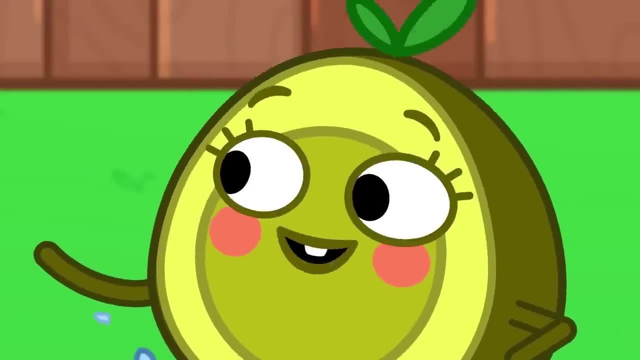 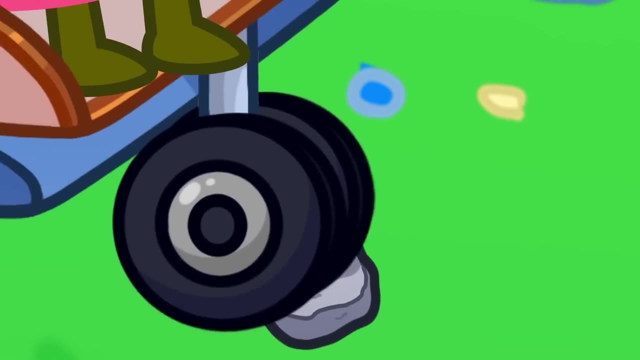 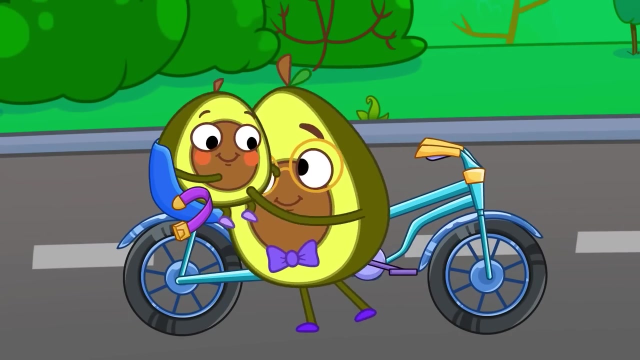 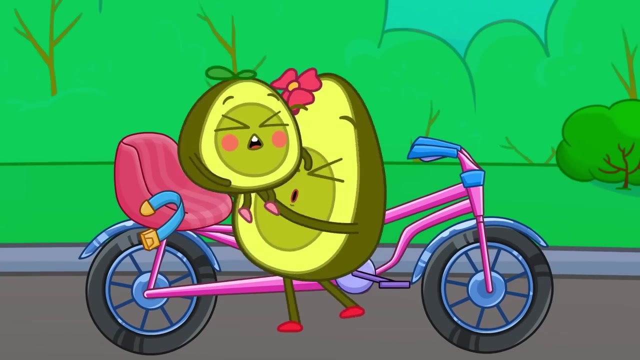 Baby lost her doll, But the seatbelt kept Baby safe. Buckling up seatbelts is very important. Ah, The seatbelt is protecting Baby and her doll. Okay, Pit, Don't forget your seatbelt and your helmet. You too, Penny. 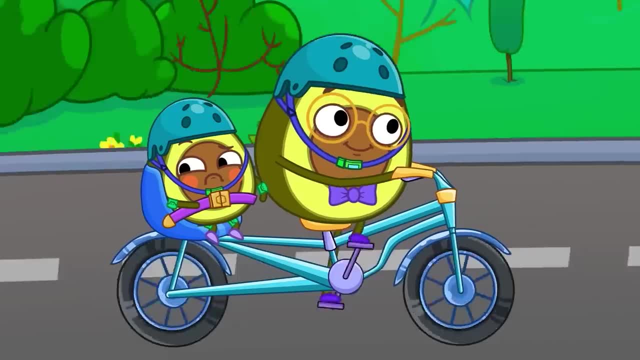 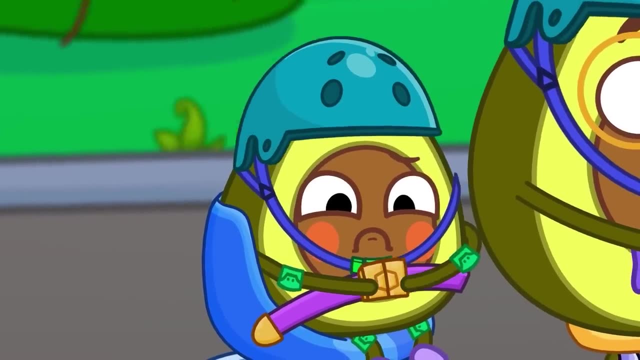 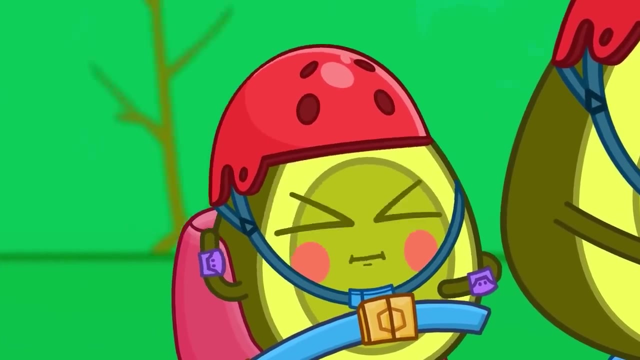 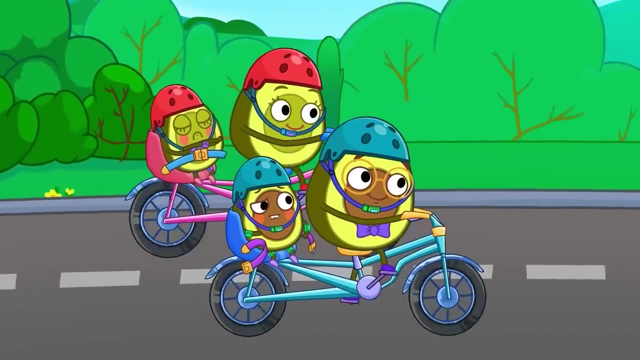 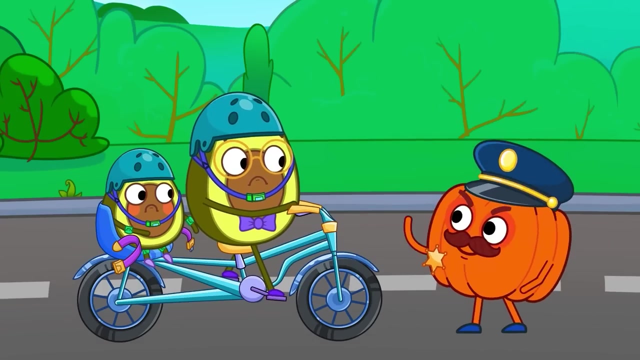 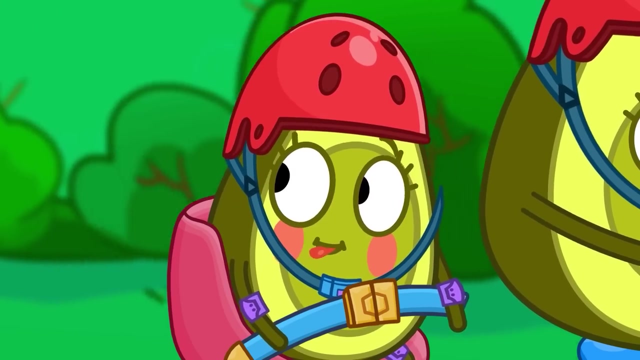 Pit wants to unbuckle his seatbelt. Oh, Pit, Pit, buckle up your seatbelt, Pit doesn't want to. Ta-da, Officer Pumpkin wants Daddy to stop. Oh, Oh, Uh-oh, Hehe, Uh-oh. 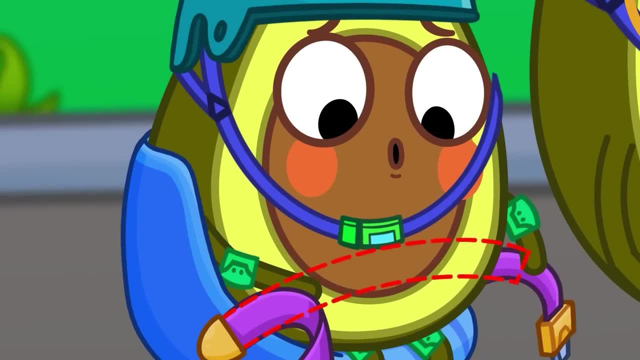 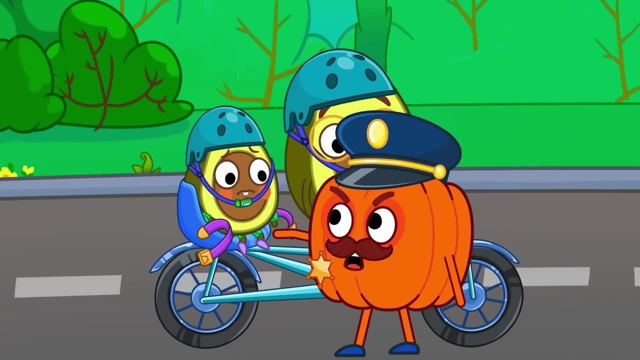 Uh-oh, Uh-oh, Uh-oh, Uh-oh, Uh-oh. Pit needs to buckle up. Huh, Huh, Uh-oh, Uh-oh, Uh-oh. Seatbelts are very important. 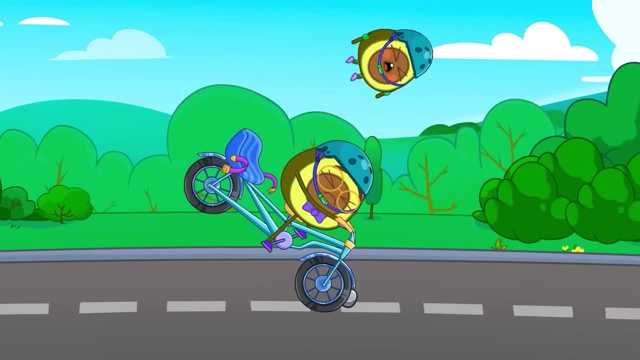 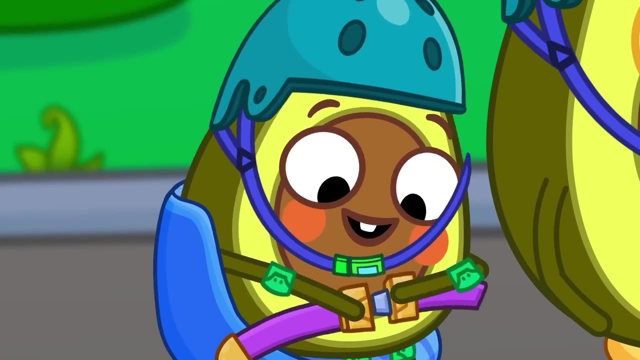 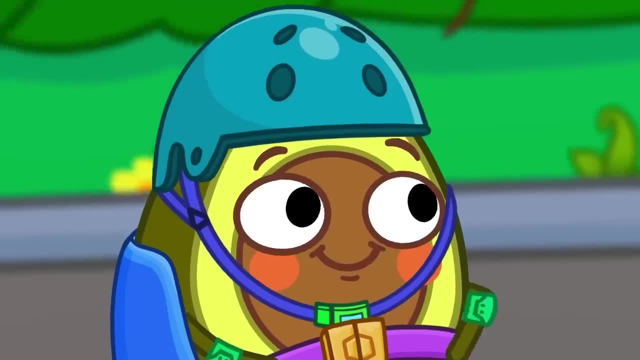 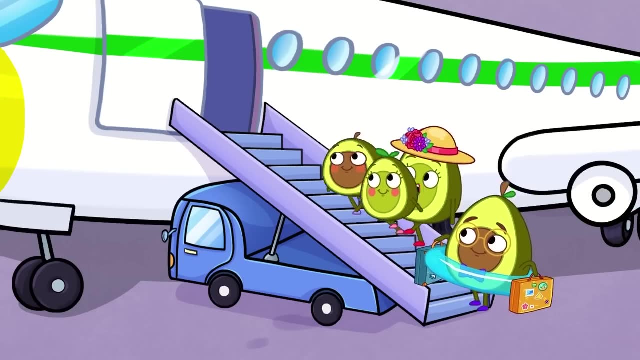 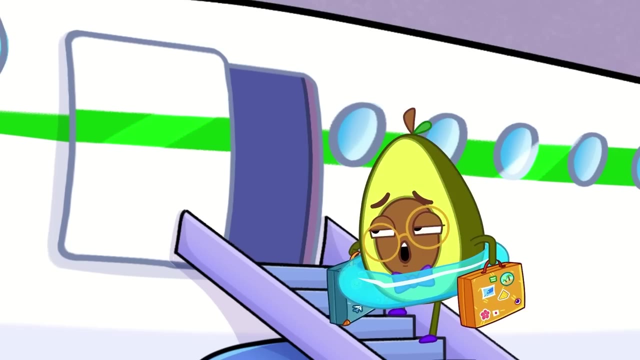 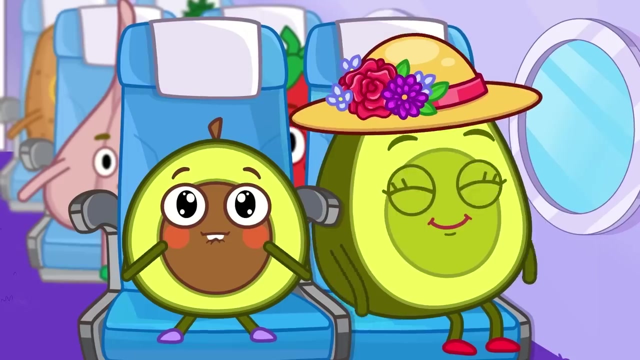 Uh-oh, Enjoy your bike ride, kids, Kids, we are going on a trip. Hooray Pit and Penny are going on vacation. Hurry up, Daddy, The airplane will leave soon. What are you going to do on the plane, Pit? 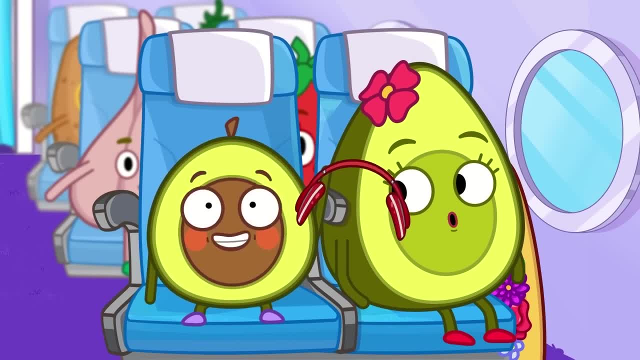 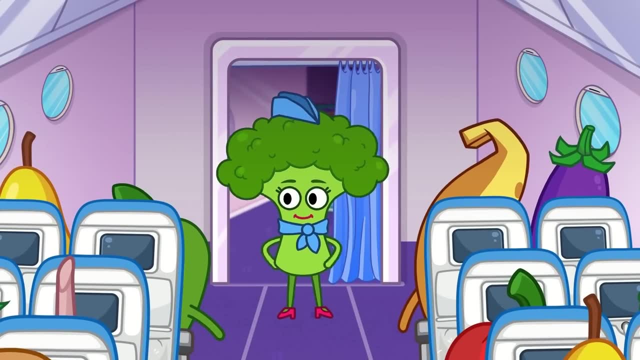 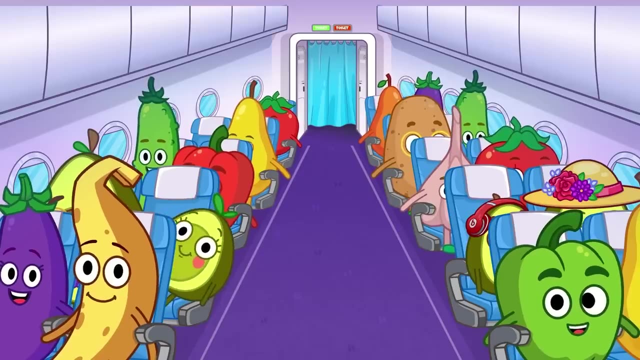 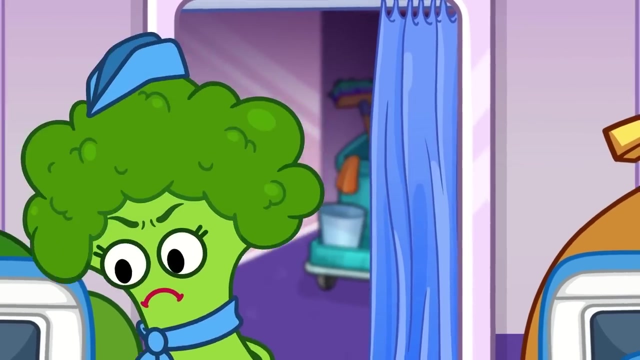 I'm gonna listen to my music for the whole flight. This is the flight attendant and she has an announcement. Hello, dear passengers, Please listen to the safety rules. Pit, Pit, Oh no, Pit's music is too loud. Why not tap him on the shoulder? 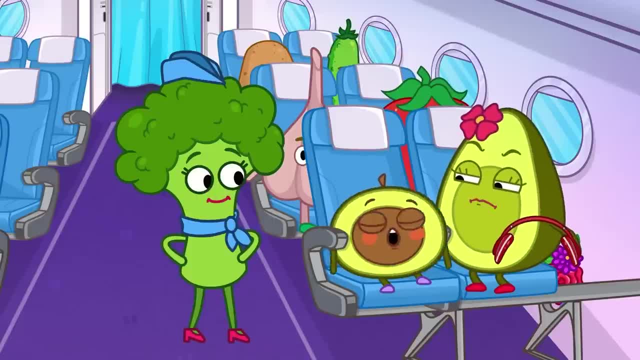 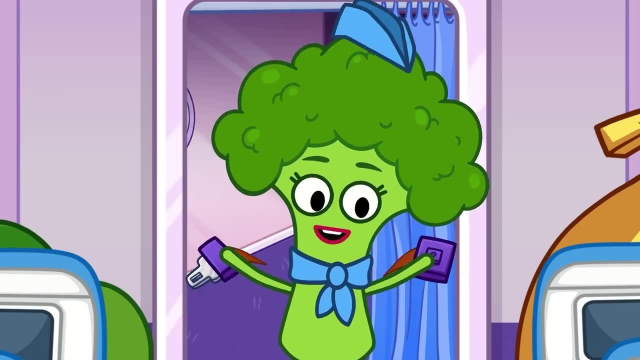 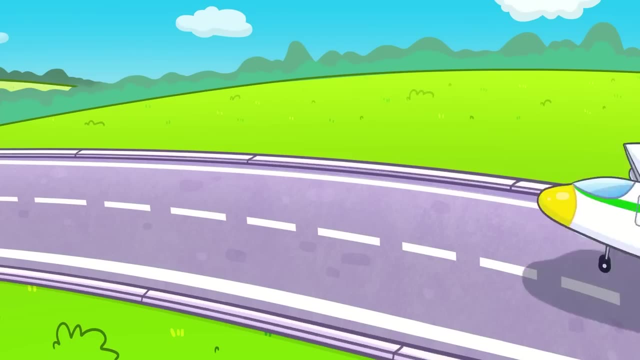 Pit, You need to listen to the safety rules. Okay, I'm sorry. It's okay, Pit is ready to listen. Please fasten your seatbelts. It is now safe for the airplane to take off. Whee, This sign means you must stay in your seat. 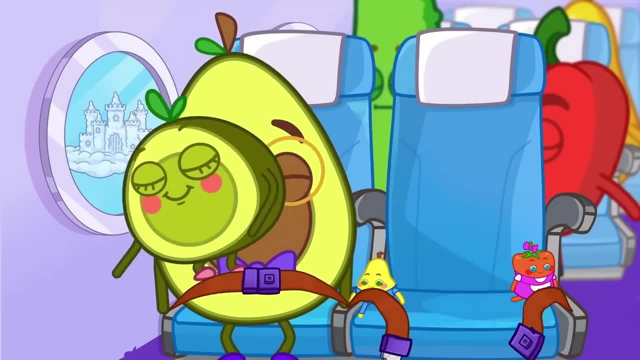 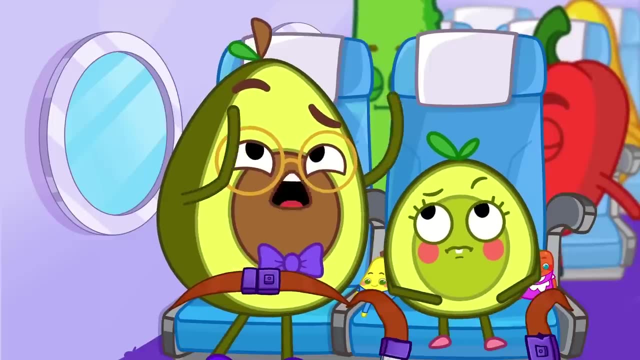 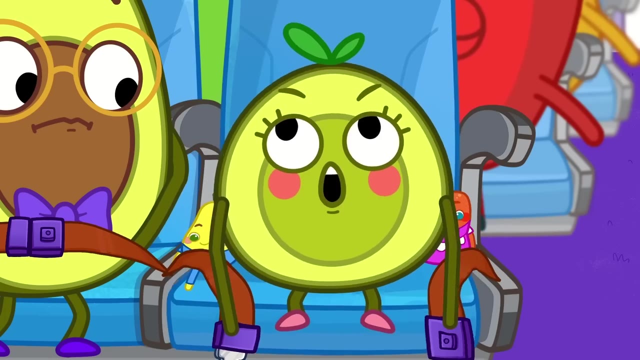 That cloud looks like a castle. Oh Penny, you've forgotten the safety rules. Oh Penny, you can't move right now. Look at this sign: You must stay in your seat when it's on. Oh, okay, Good. 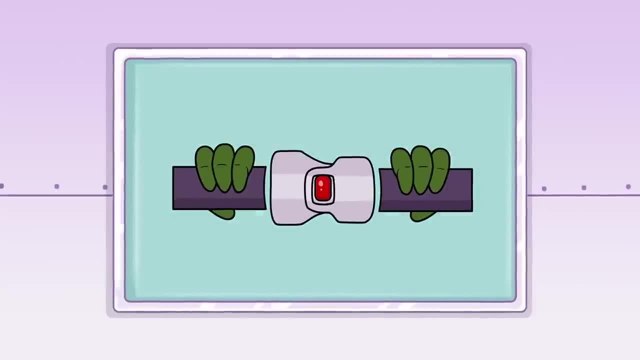 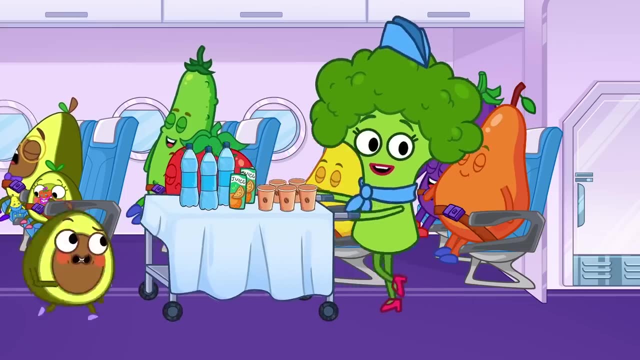 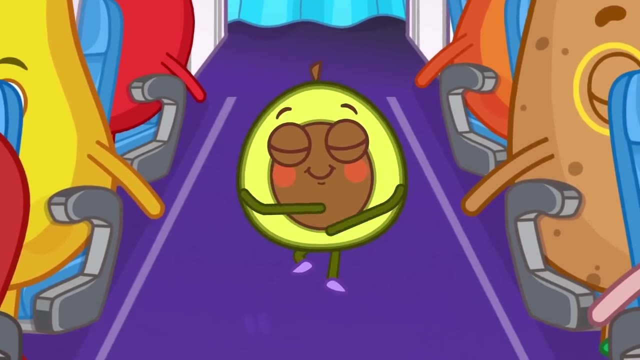 Pit really needs to use the bathroom. Hold on, Pit. Okay, Pit, You can now leave your seat But watch for others. Oops, I'm sorry, Pit, You can't run in the airplane, Do you understand me? Yes, Mommy. 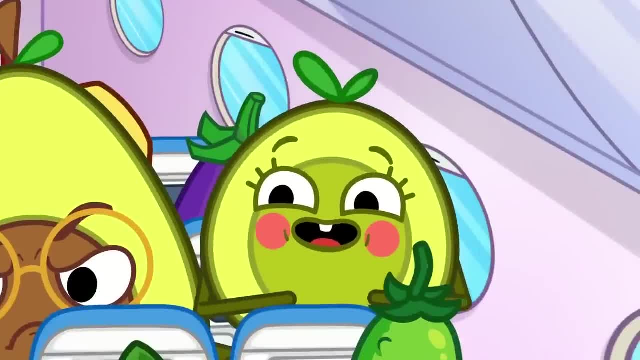 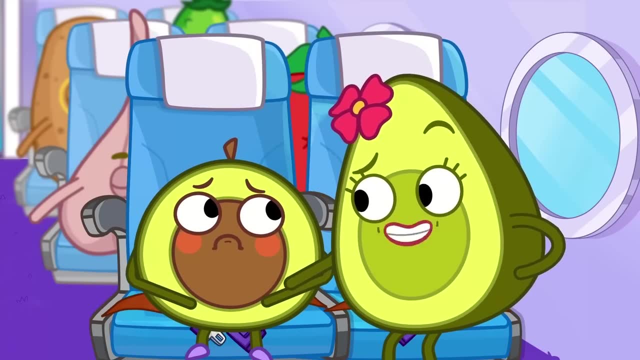 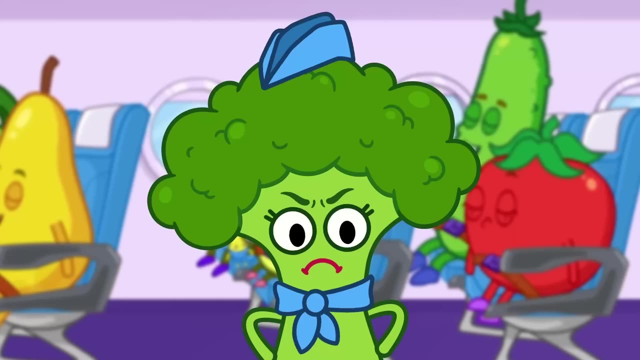 Okay, I'm sorry. What's wrong? Oh, it's okay, Pit, you can't run in the airplane, Do you understand me? Yes, Mommy, Okay. Okay, here you go. Time to put your seatbelts back on. 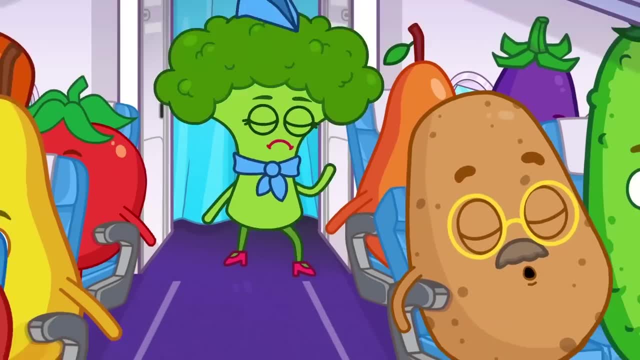 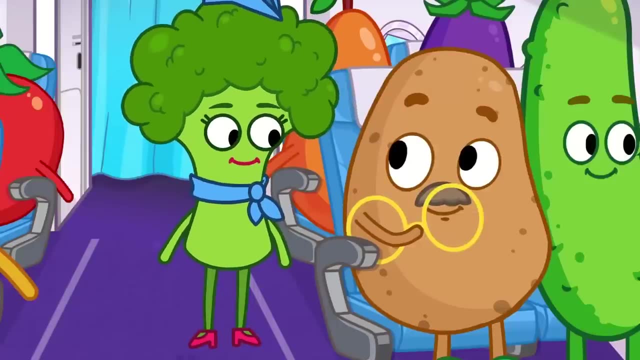 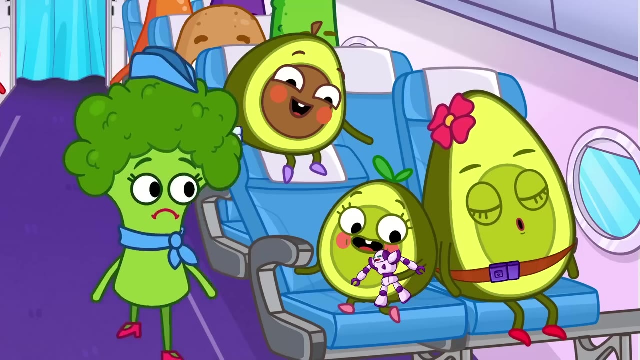 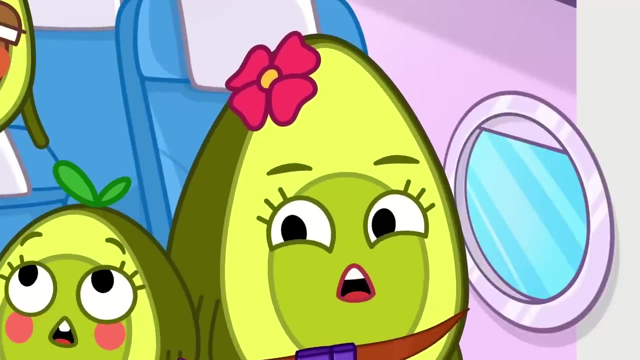 Yes, Mr Potato, that means you too. Oh, I'm sorry. Thank you, sir. What are Pit and Penny up to now? Ahem, ahem, Wake up, Mommy, What They are being too loud. 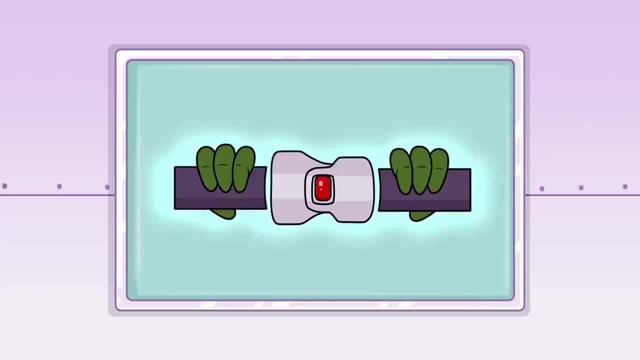 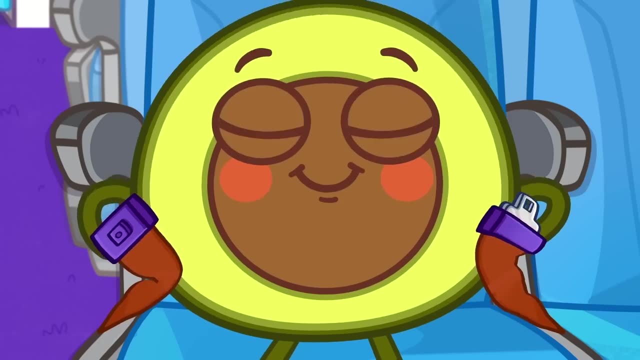 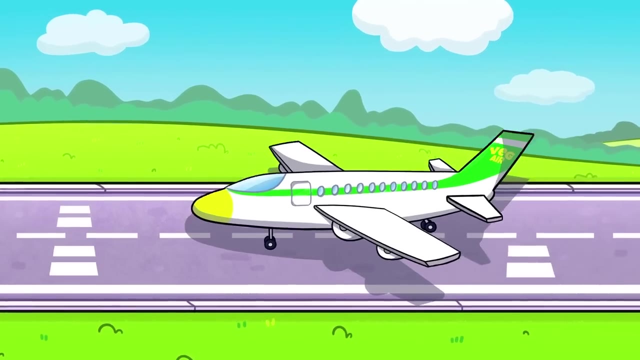 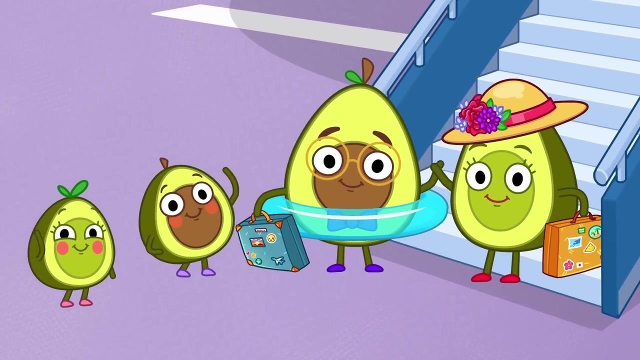 Kids be quiet. Oops, we're sorry. Penny returns to her seat And Pit buckles up his seatbelts. There we go, And now the flight is over. Bye, Pit and Penny, and Mommy and Daddy, Have a nice trip. 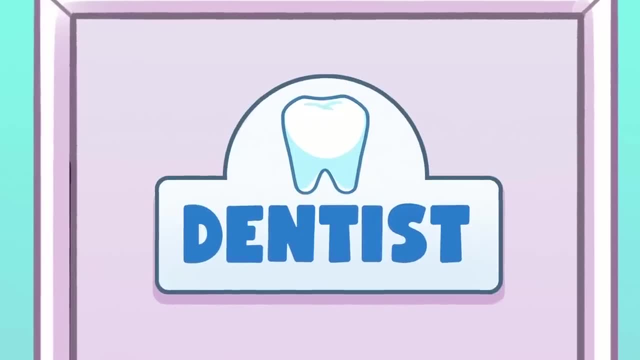 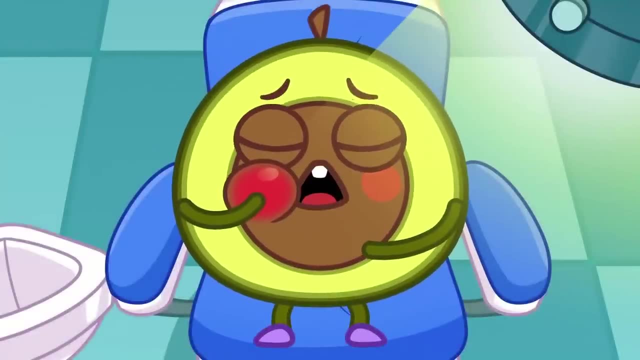 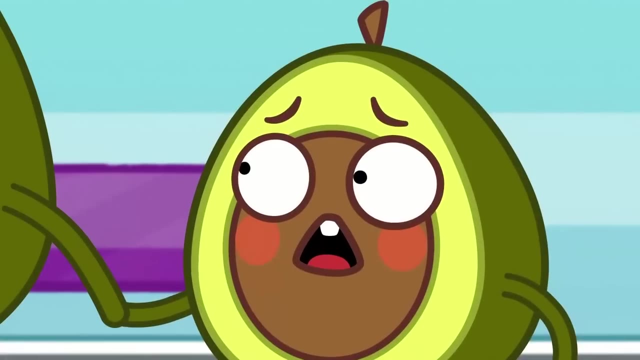 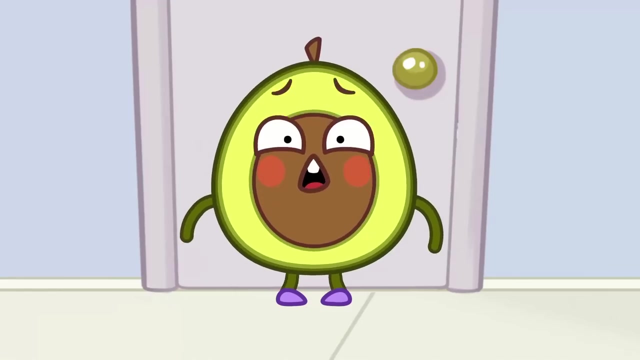 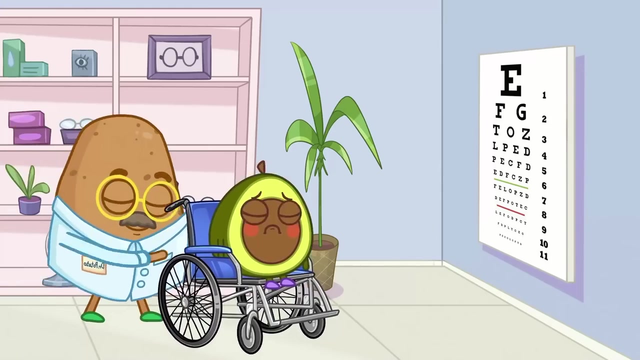 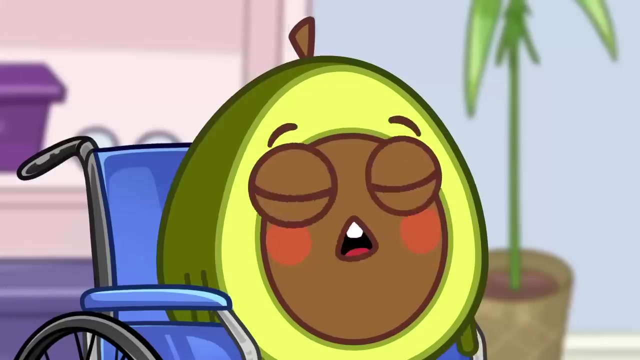 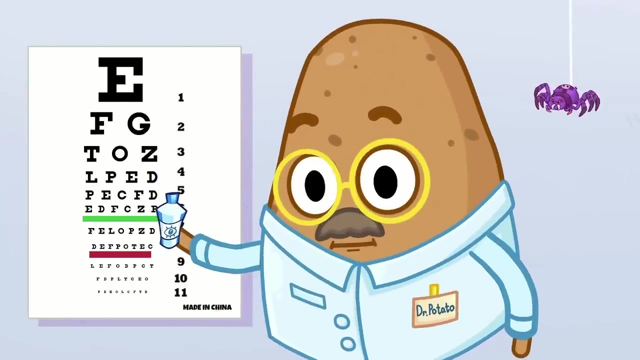 What's wrong, Pit? Oh, you have a dentist appointment. Pit thinks dentists are scary. He ran into an eye doctor's office. Can you read the eye chart, Pit? Oh, you have bad eyesight. How about it? 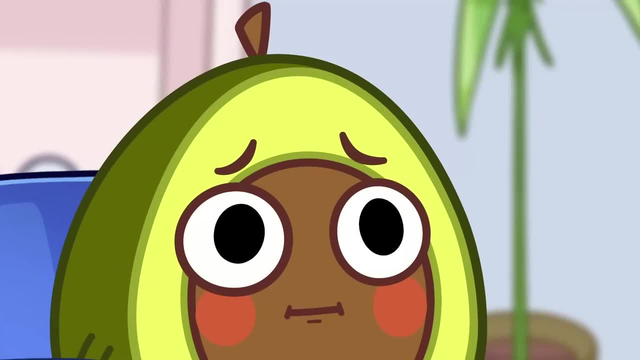 Hmm, Did you know that you can't even see? Yeah, At least you're the one who knows. Now I'm going to make you go to school. Now I'll go see my dad. Daddy, I'm out of here. 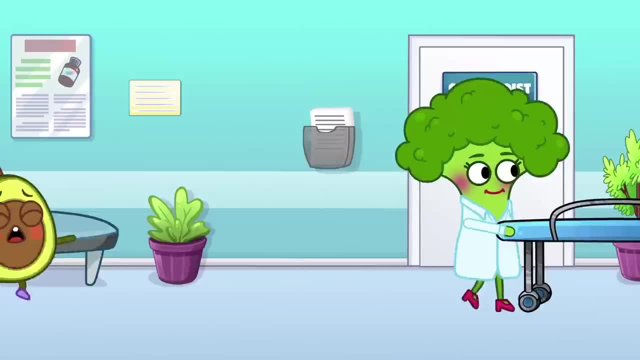 Why don't you come with me? Yeah, I should come along. You're going to be a really good teacher. I can't wait for you to make your school. Hey, little sister, Have some coffee. I'm gonna bring it over. 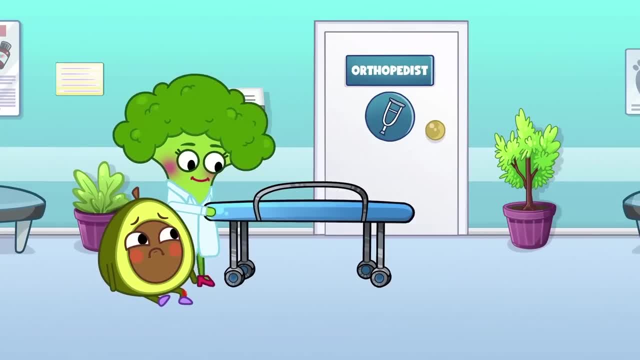 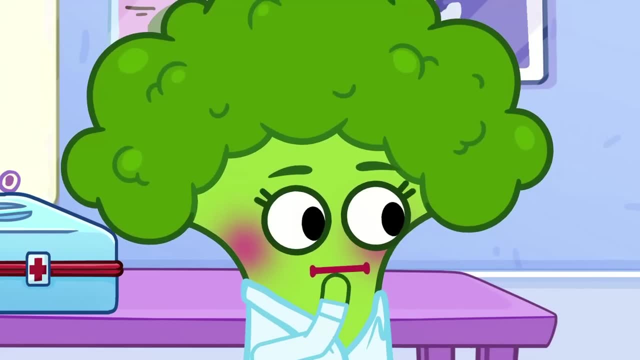 I hope you have a bird, Especially for kids. Come on, Let's go. Who'll be coming today? I'm excited. Who's going to be there? We're going to see your dad Come with us. Yeah, Okay, bye-bye. 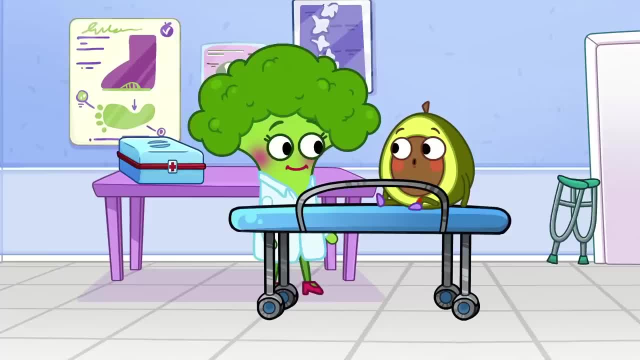 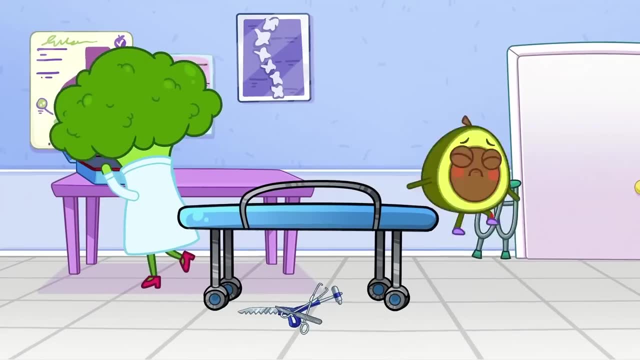 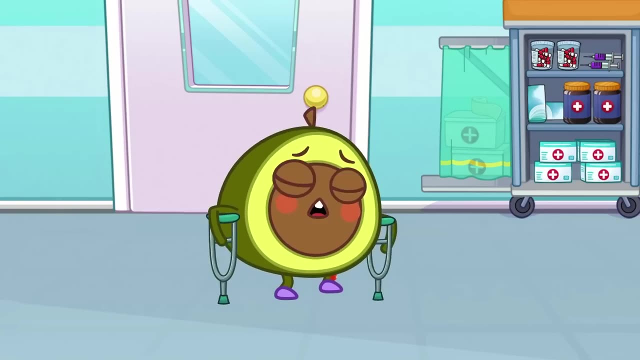 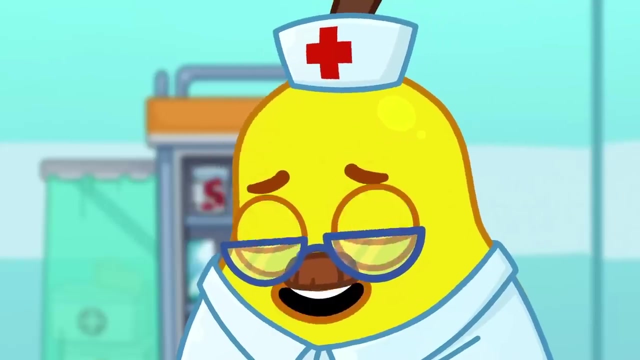 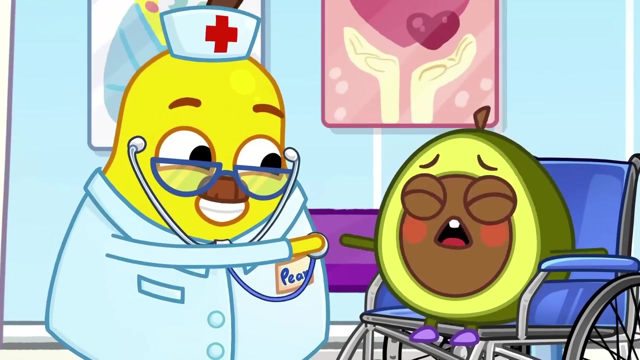 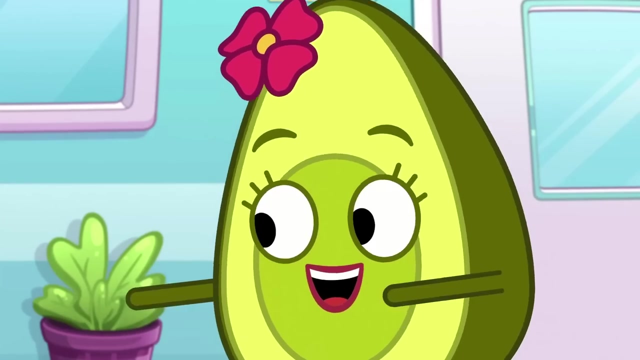 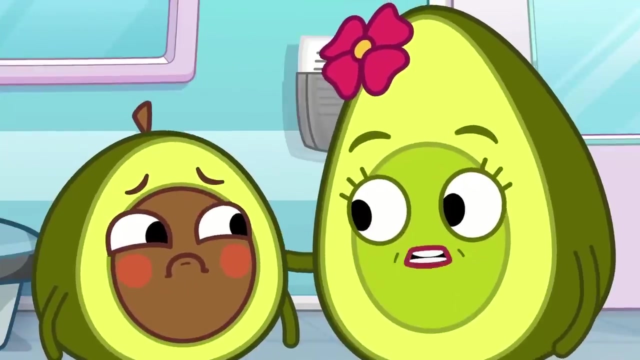 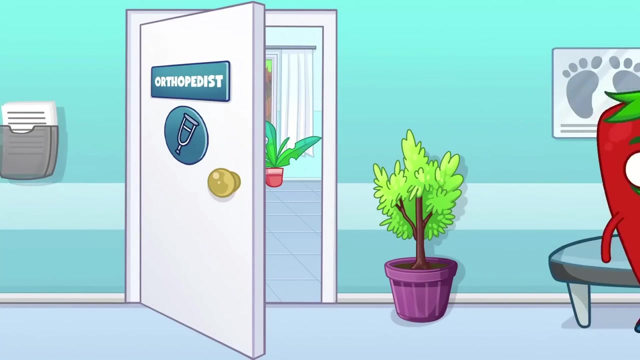 See you tomorrow. kids, you ran away again. here's another doctor. oh no, he urgently needs help. tell mommy what's wrong. pet, there are scary doctors everywhere. don't be afraid of the doctors. they help us. orthopedist treats our bones. the ophthalmologist treats our eyes. 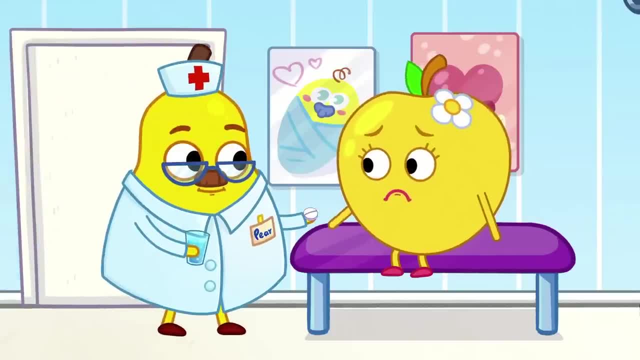 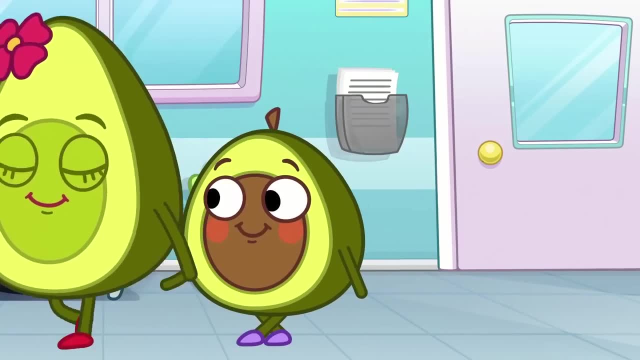 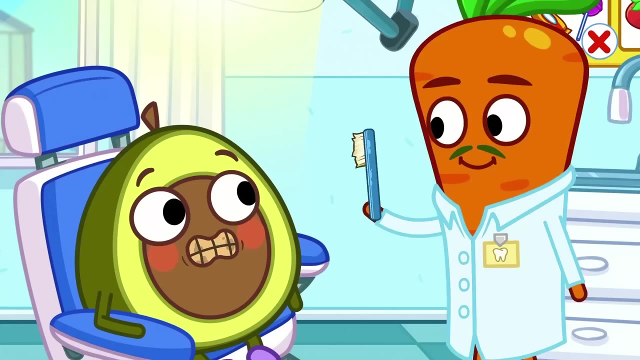 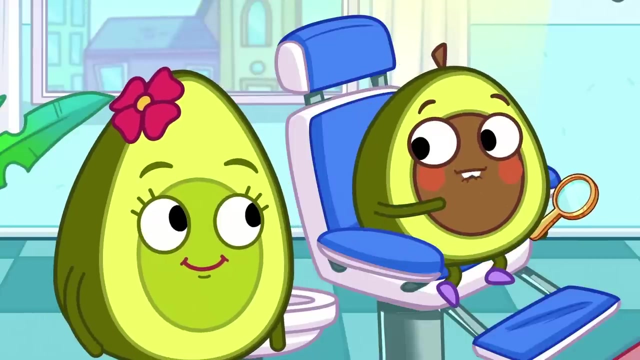 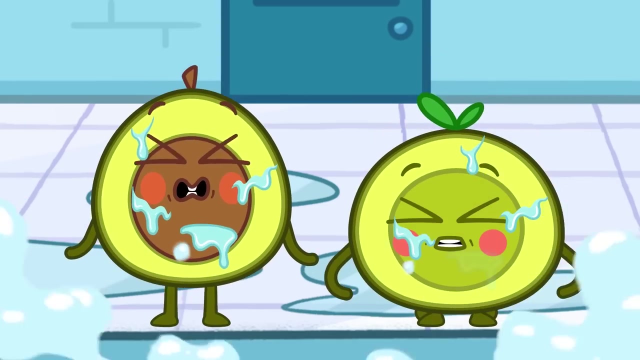 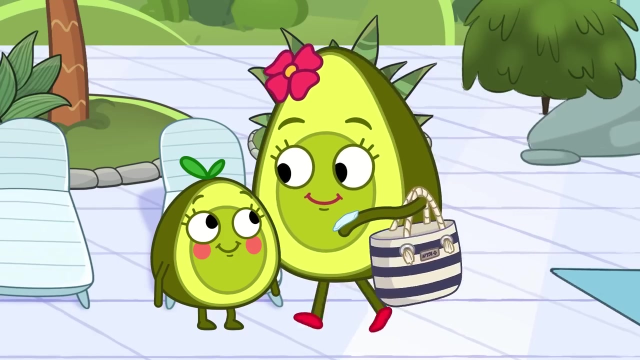 what does dr pear do? a cardiologist treats our hearts. and don't forget the dentist. he helps make your teeth clean and healthy. i'll never be afraid of doctors anymore. that's great pit. watch out bit and penny, don't be upset, it's just water. before you play outside, always put on sunscreen. 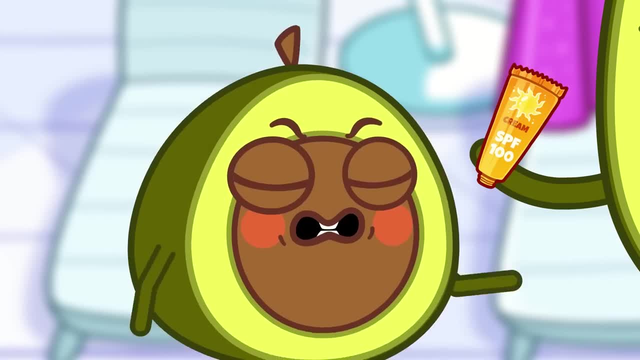 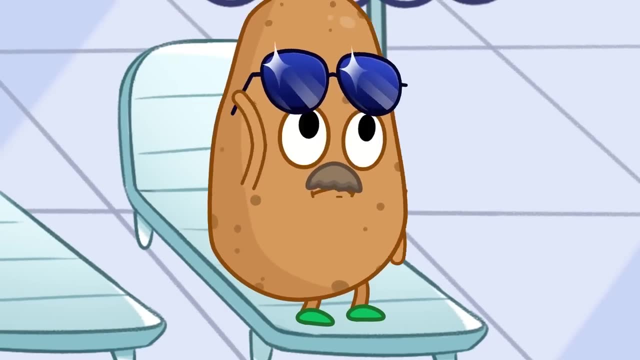 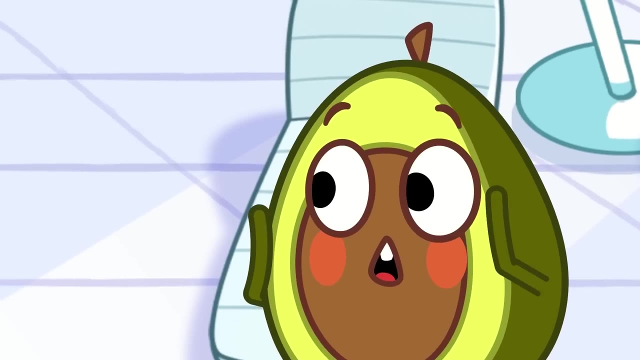 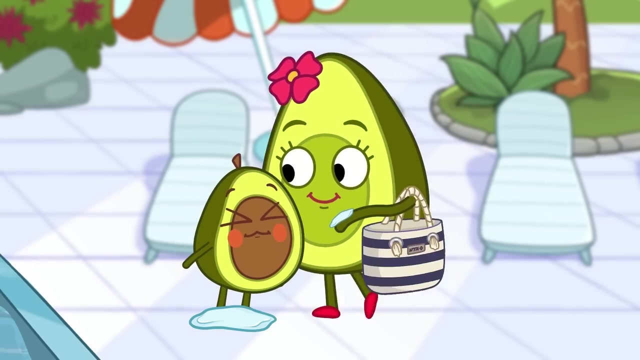 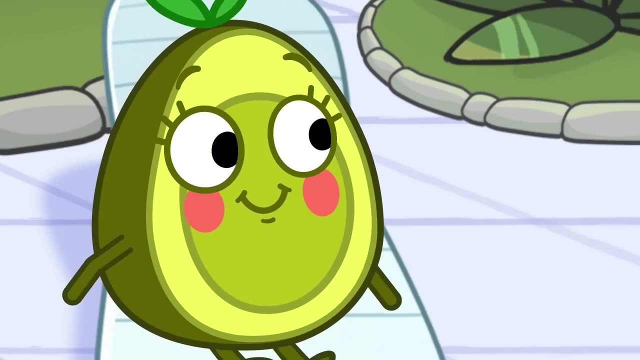 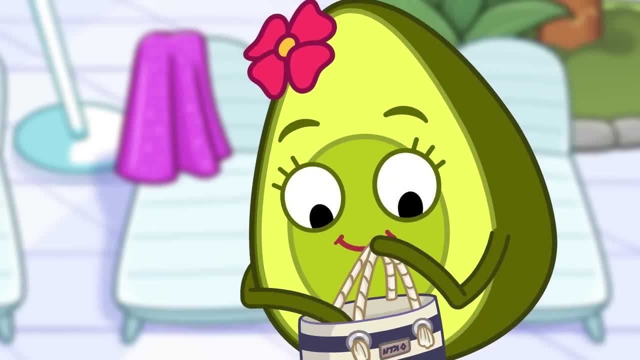 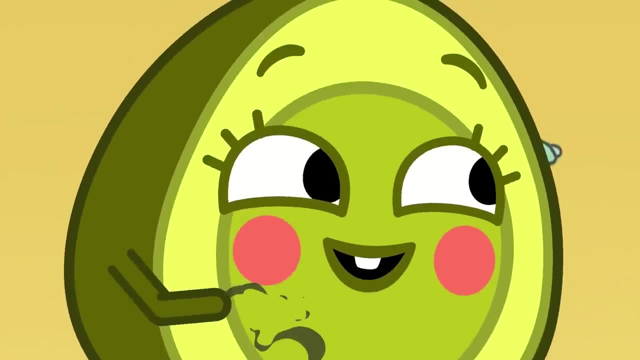 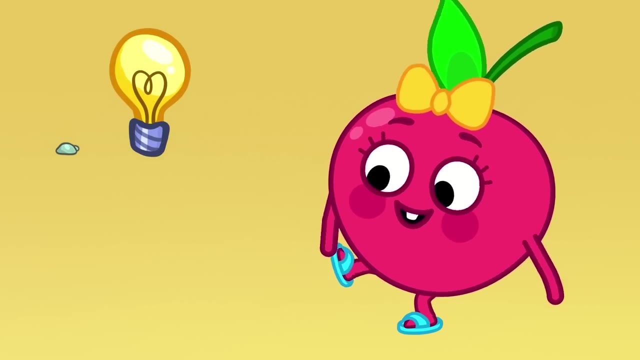 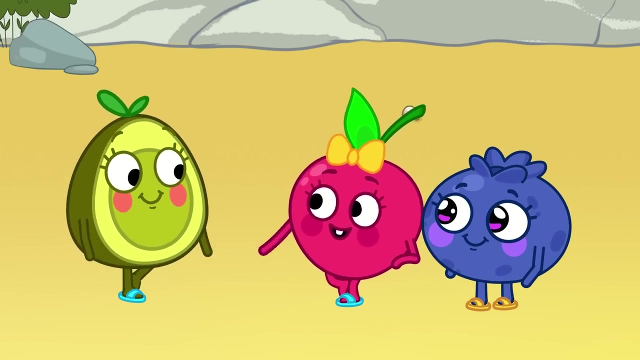 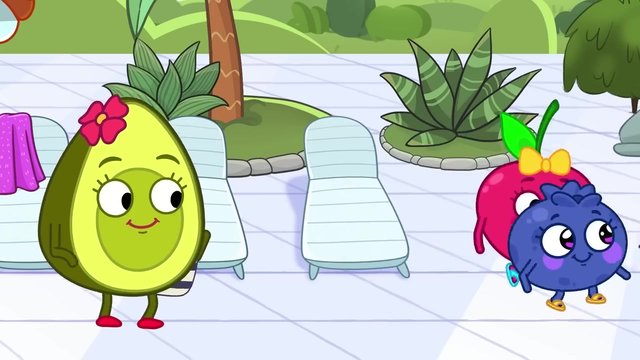 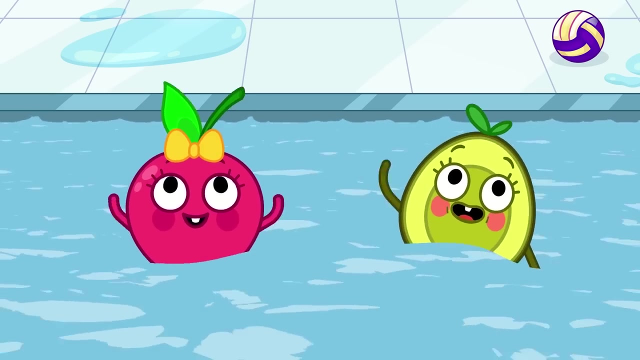 mommy also brought flip-flops to wear. oh, oh, careful, penny, that sand is very hot. maybe her friends can help. maybe one flip-flop is better than none. oh oh, one flip-flop is better than none. one flip-flop is better than none. What's wrong? Blue? 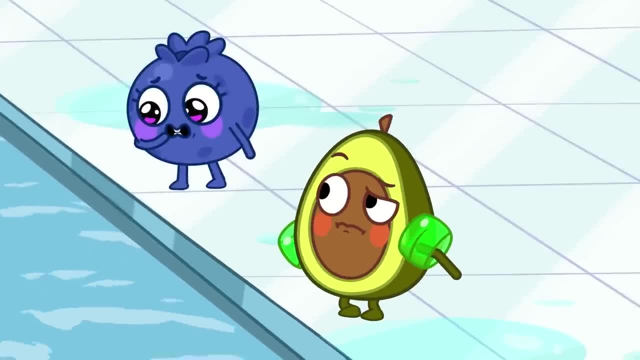 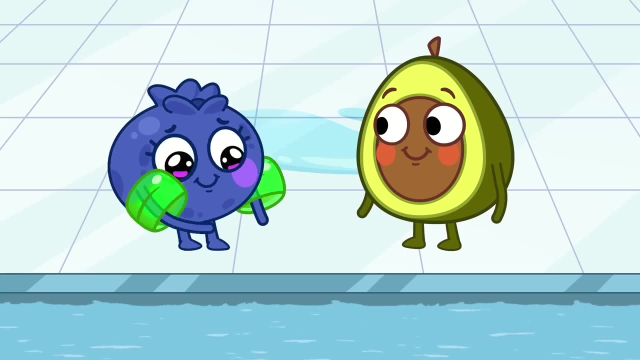 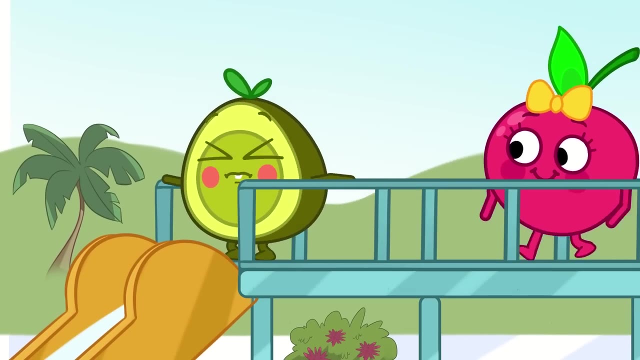 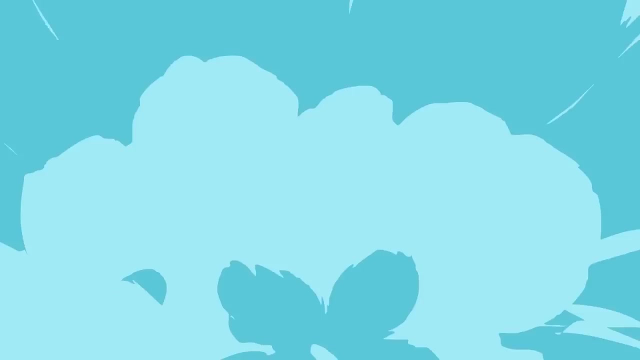 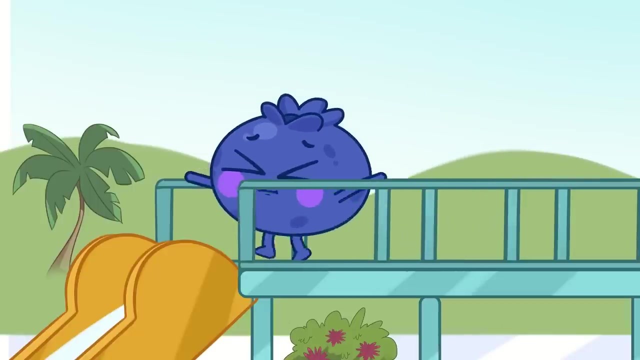 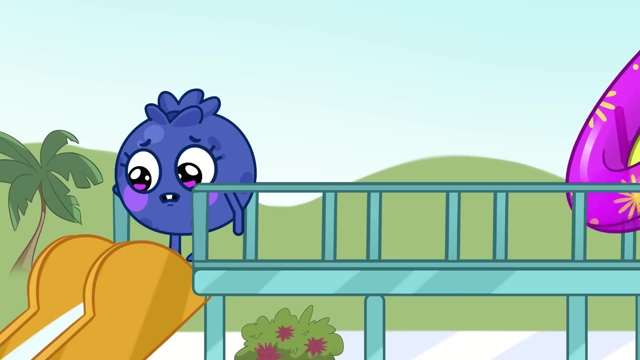 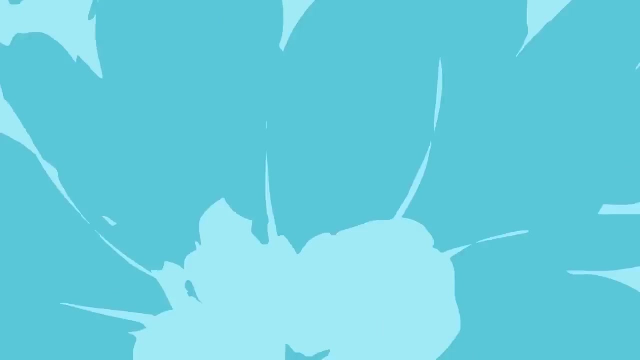 Pit. Blue is afraid of the water. Pit knows what to do. The water slide looks very tall. Don't be scared, Penny. It's now Blue's turn, But Blue is also scared. Blue and Pit can go down together. What a wonderful day at the pool. 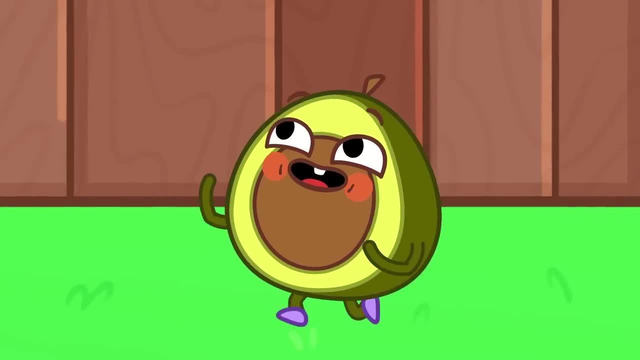 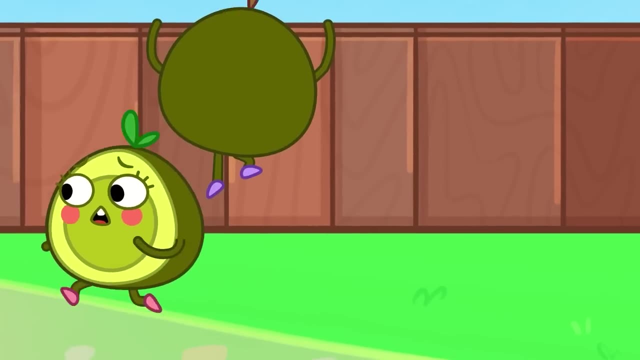 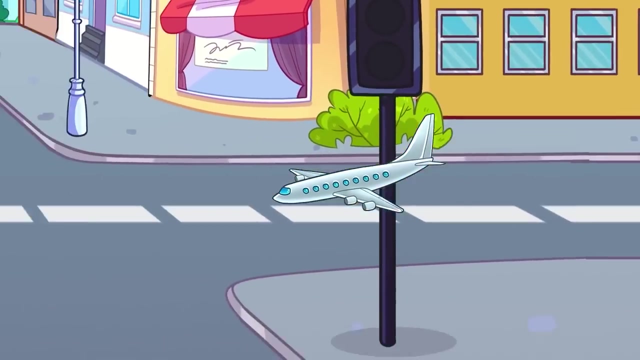 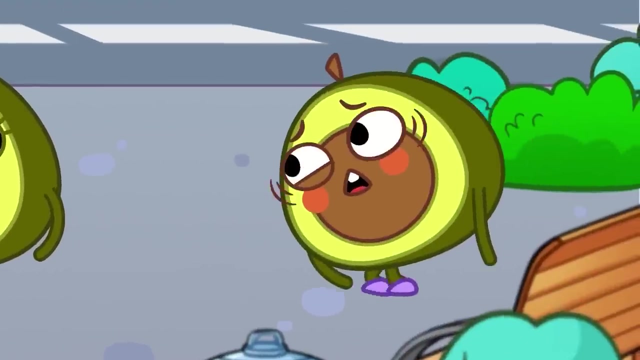 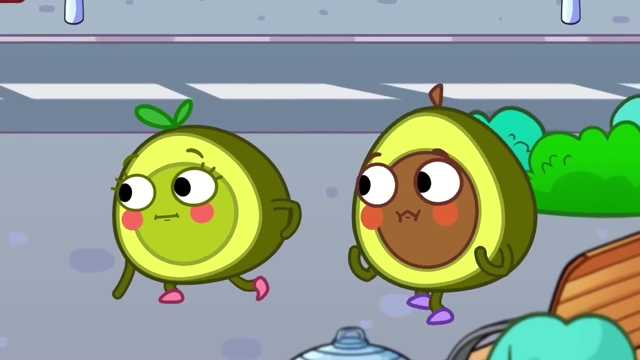 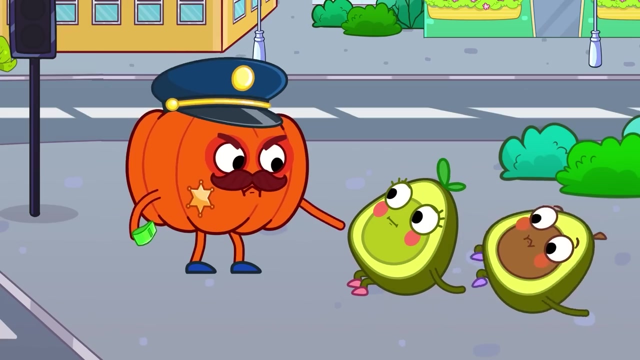 Pit and Penny are playing with their toy plane. It's gone over the fence. Go around the fence, Pit. There's the plane. It landed in the water. It's in the street. Stop kids. It's Officer Pumpkin. The traffic light is red. 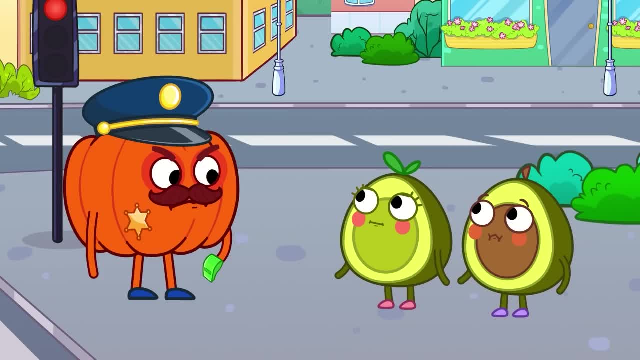 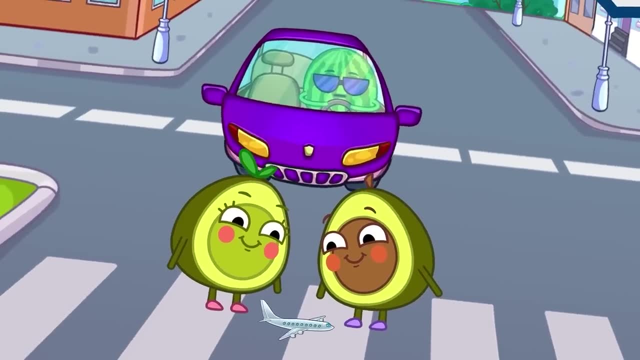 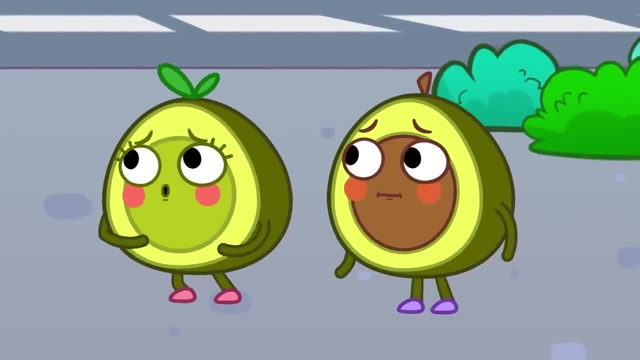 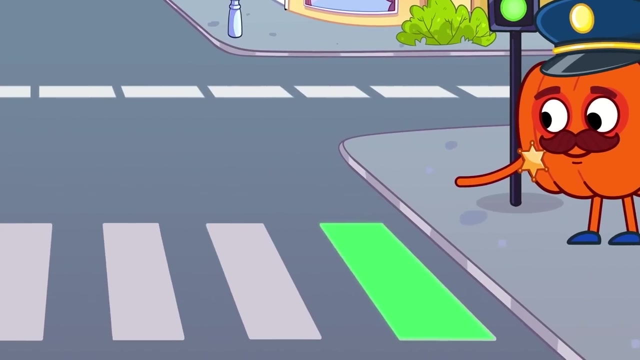 It mustn't cross the road on the red light. The road is very dangerous. You have to watch for cars. And what should we do? Here comes the green light. You can go. Green means it is safe, but Don't run. 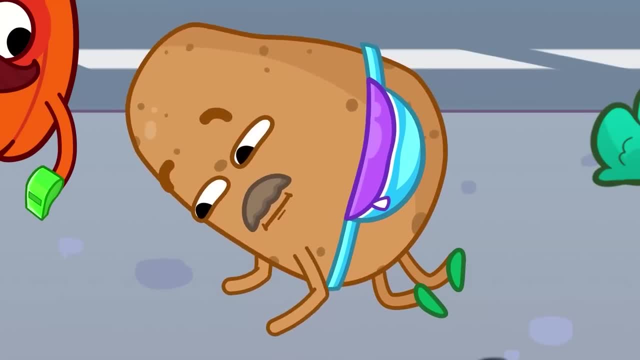 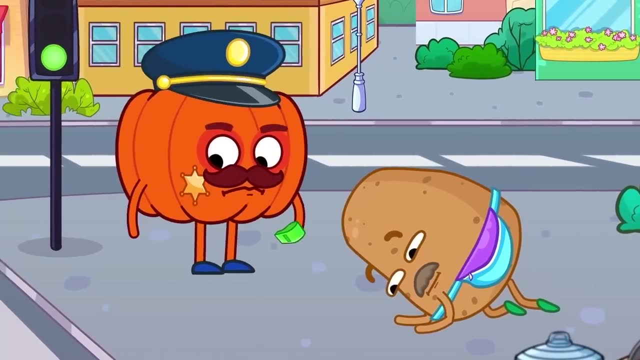 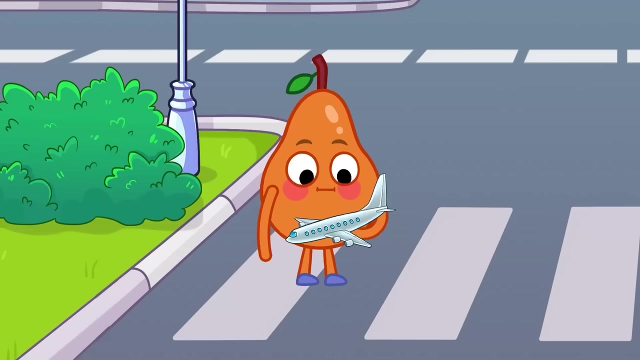 Someone else needs help. Has anyone seen my glasses? Officer Pumpkin will help find them. I'll go find them. The race is on. The race is on. Hurry, don't lose yourself. You can't come over here. I have to run. 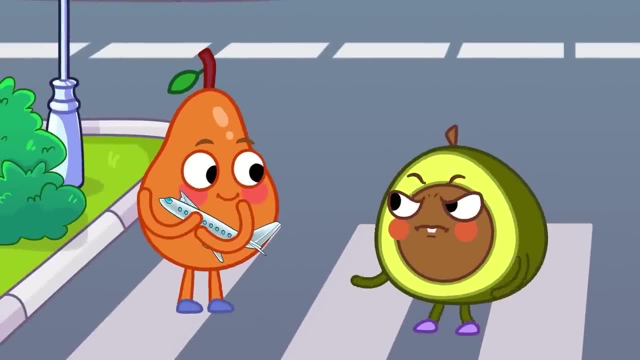 The Blue team won't let me down. Mr Sterling, you can do it. You can do it. The blue team is one step ahead. It looks like they're going to hit us again. Let's run, I'm going to take it. 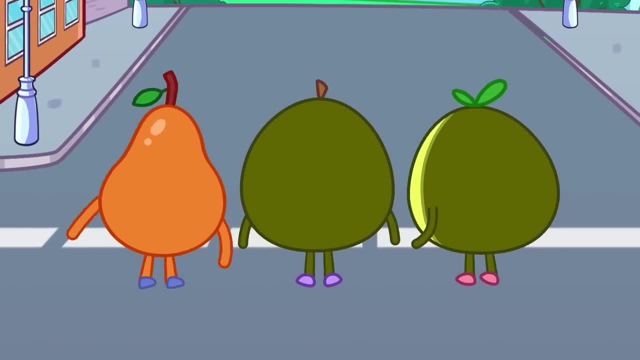 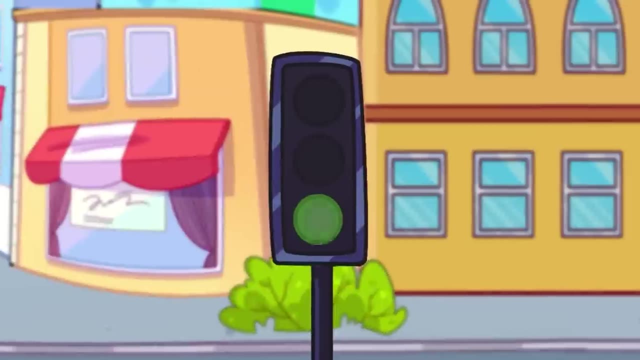 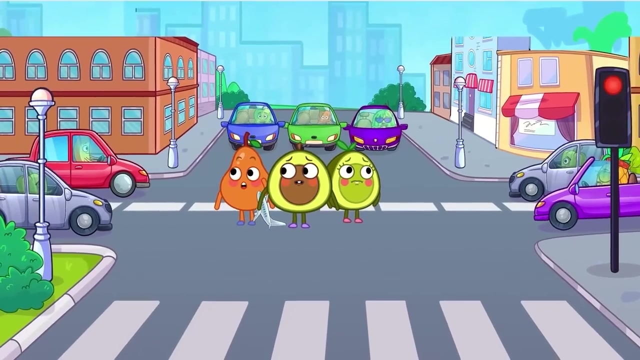 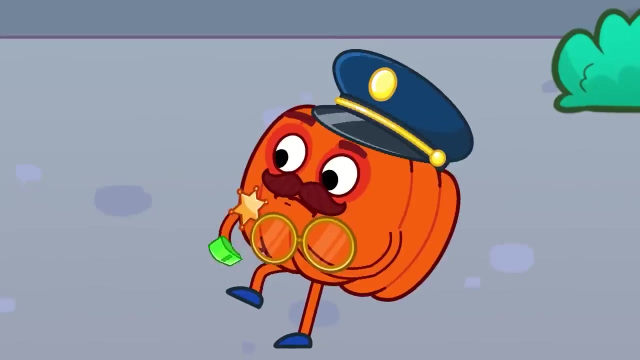 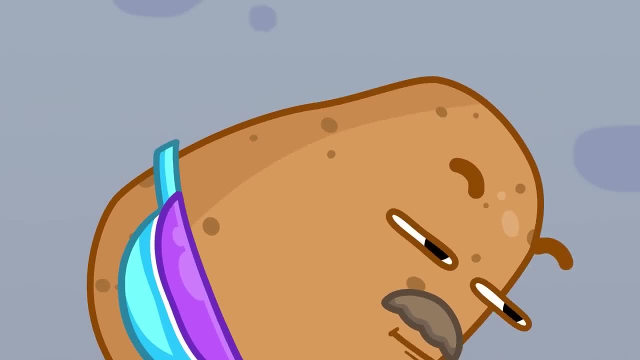 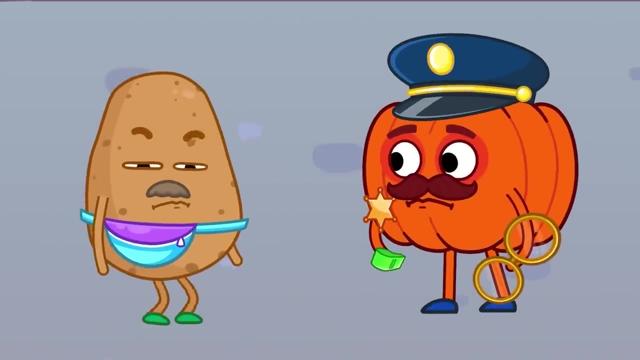 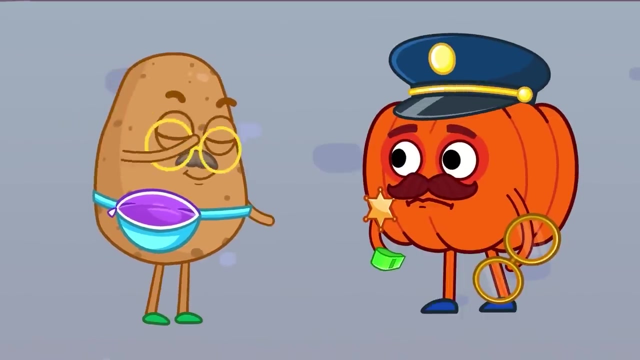 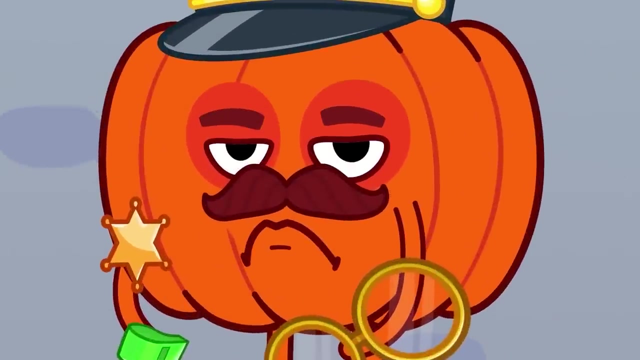 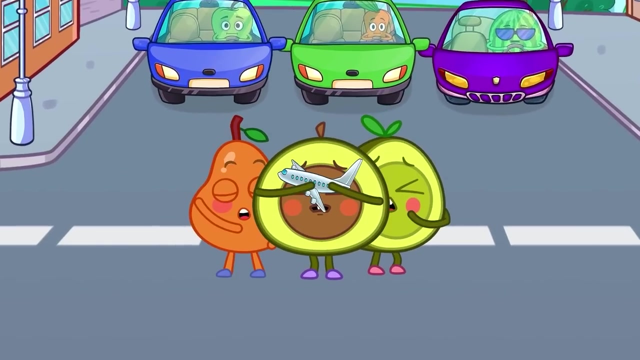 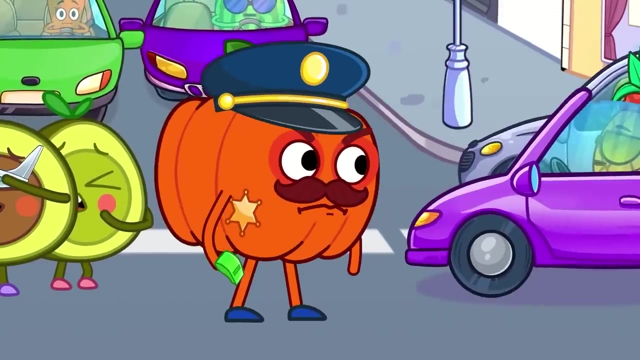 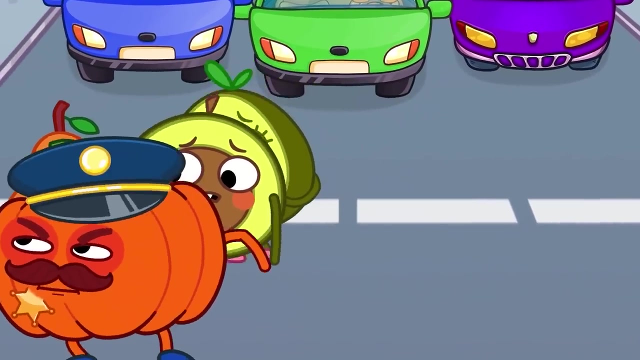 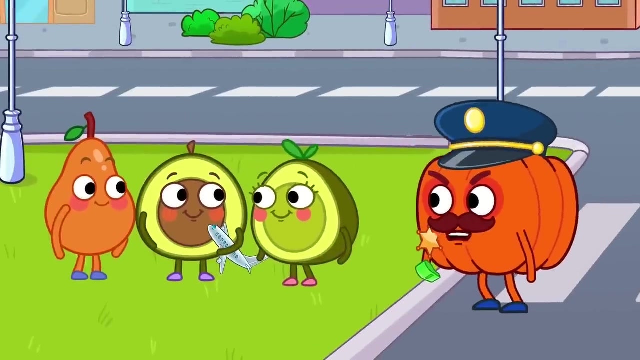 Are they yours, Mr Potato? These are not my glasses. And here are my glasses, Officer Pumpkin. The children need you. Calm down kids. Let's go Follow Officer Pumpkin. Phew, Everyone's safe Children. be careful on the road and always wait for the green light. 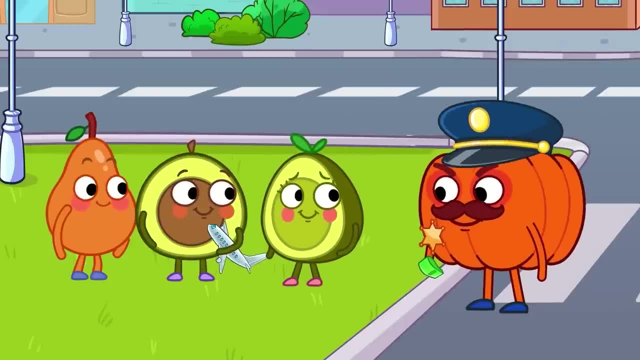 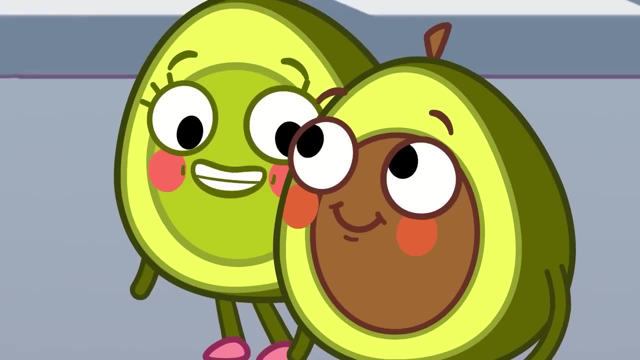 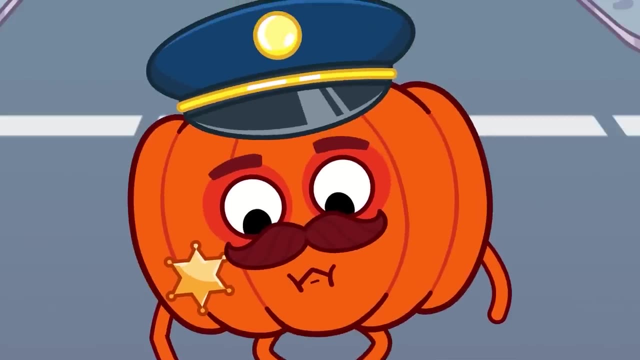 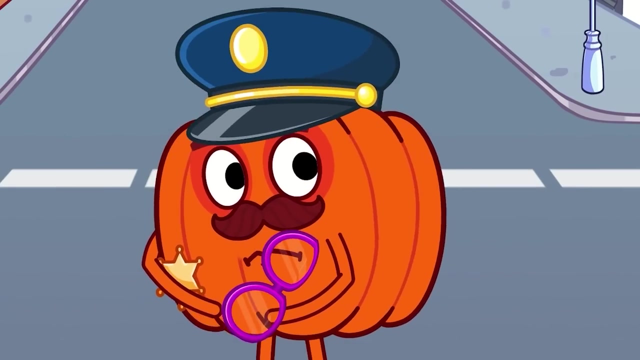 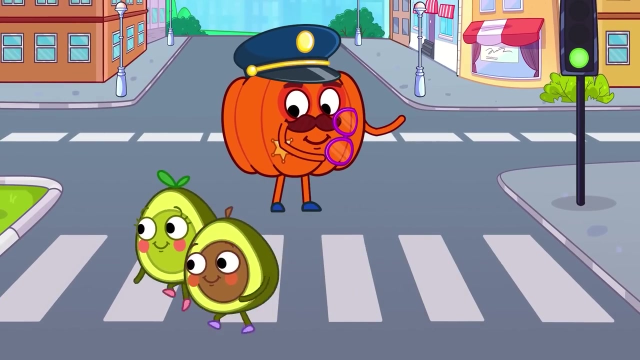 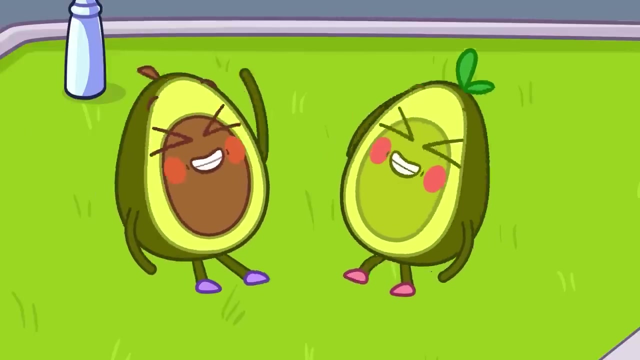 We've got it. Stop. The light is red, It's green. Let's go Pete. What's that? Hmm, Yes, We've got it. Well done, Yikes, It's the big bad wolf. There's a balloon house. 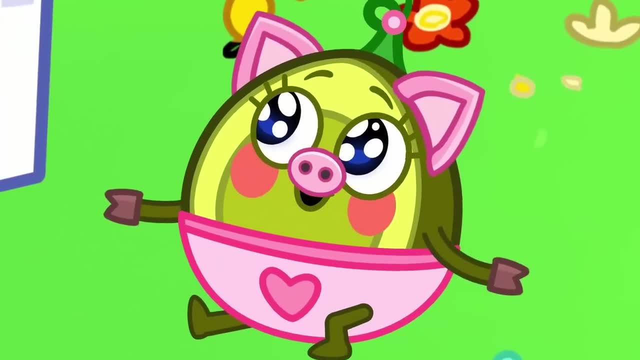 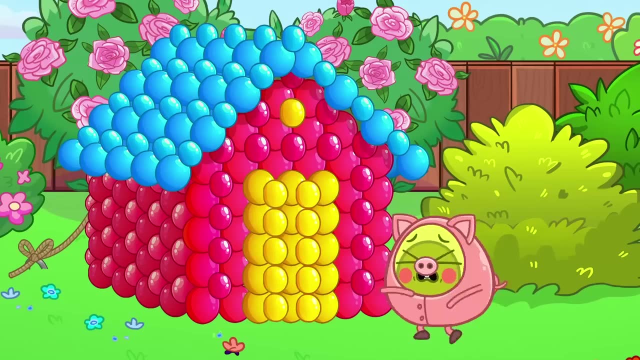 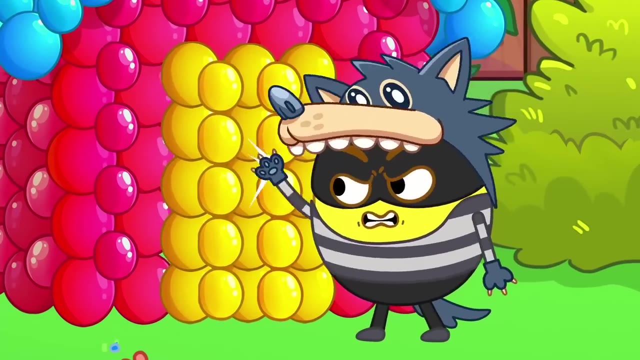 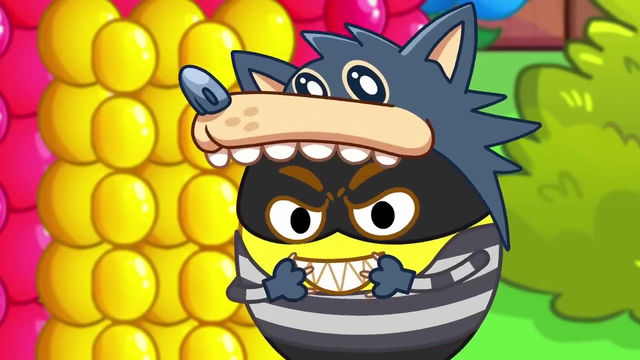 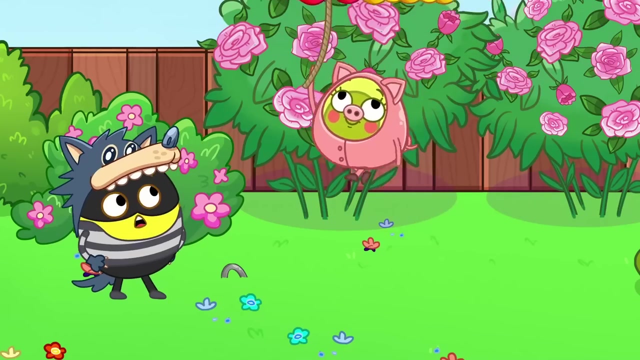 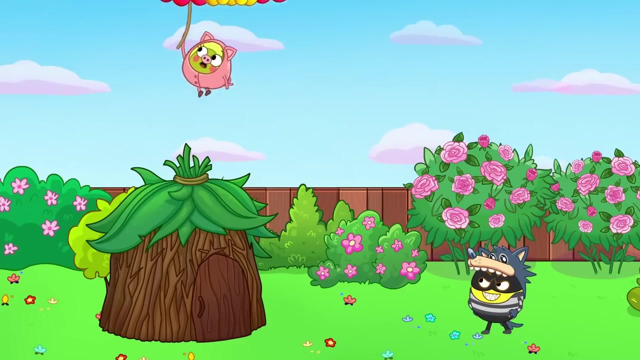 A stick house And a brick house. Yeah, Watch out, The wolf is coming. Wow, Penny, Stay inside. Huh, Huh, Huh Huh. The balloon house is floating away, But Penny is safe. Now. Pit's house is ruined. 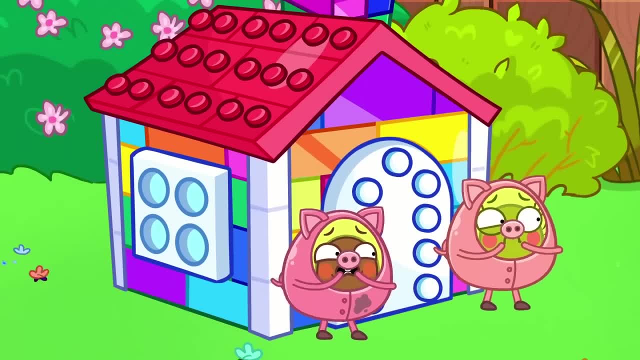 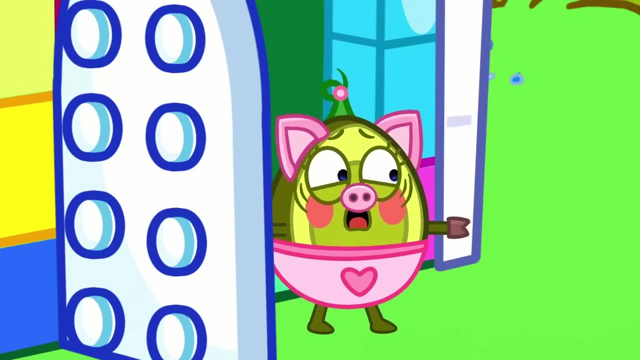 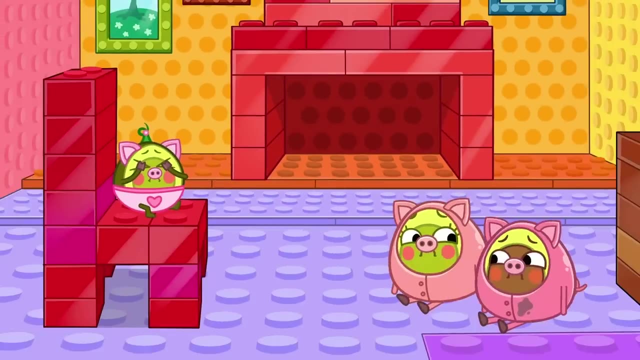 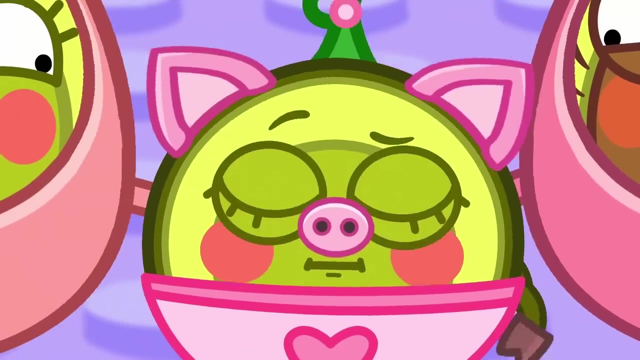 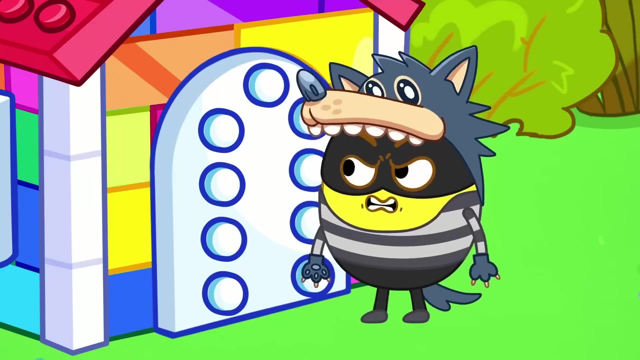 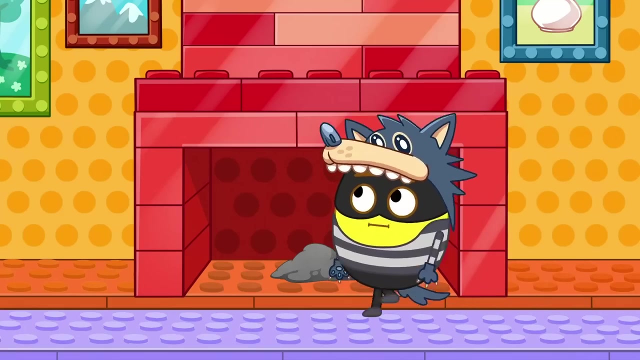 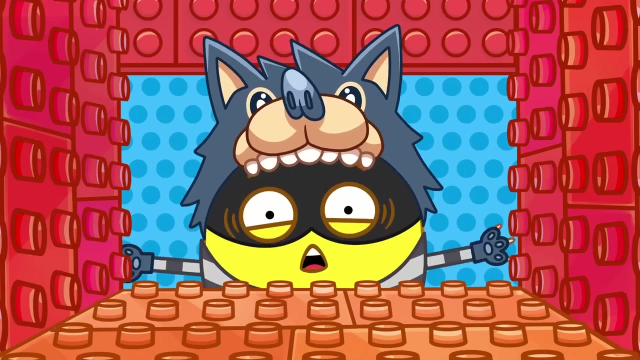 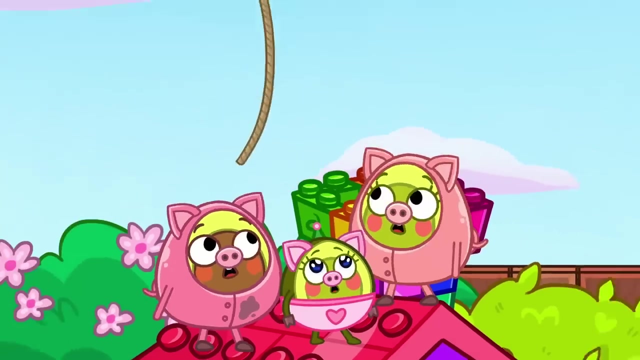 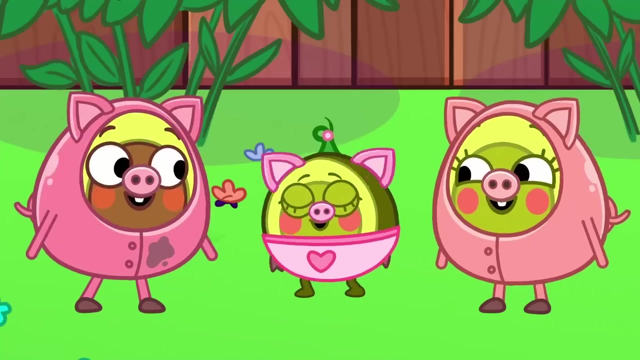 Baby Pit and Penny need your help. They'll just go down the chimney. Baby knows what to do. Where did everyone go? They're on the roof Now. Pit has an idea. I'm so sorry, I won't do it again. 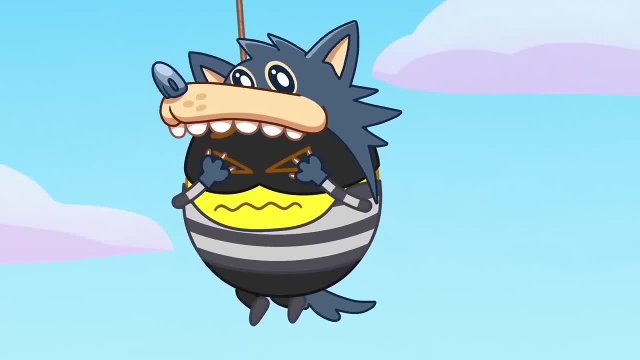 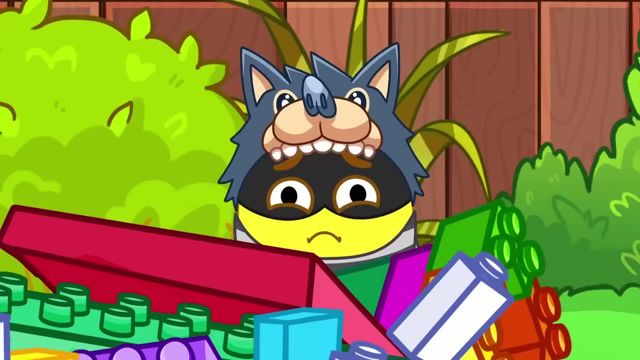 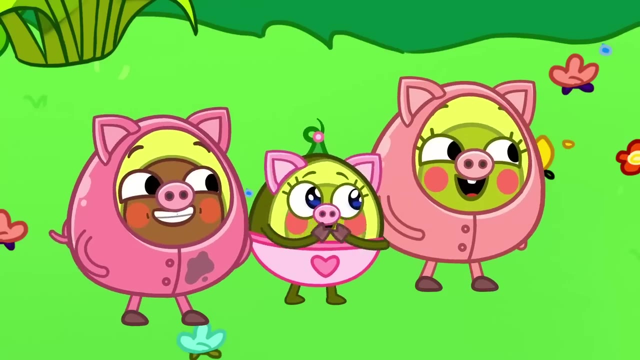 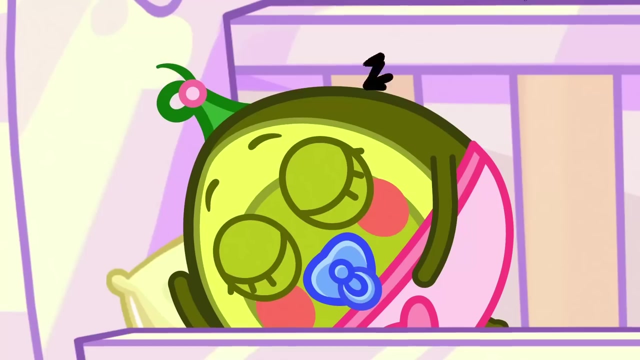 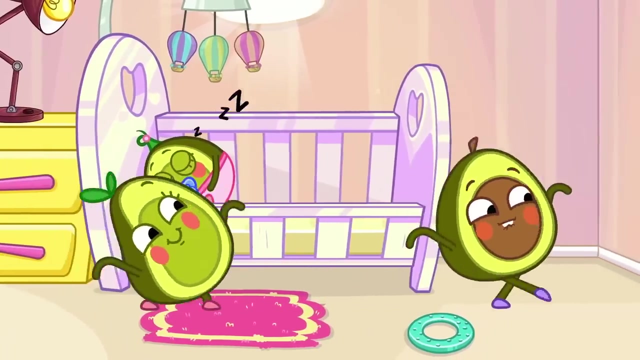 Help get the bad wolf down. Oh no, Baby's house is broken. Mr Wolf made a better house And they lived alone and happily ever after. Shh Baby is sleeping. Shh Night-night baby. Look at all the amazing food. 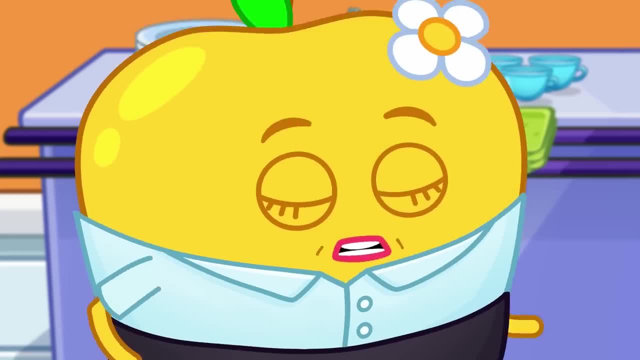 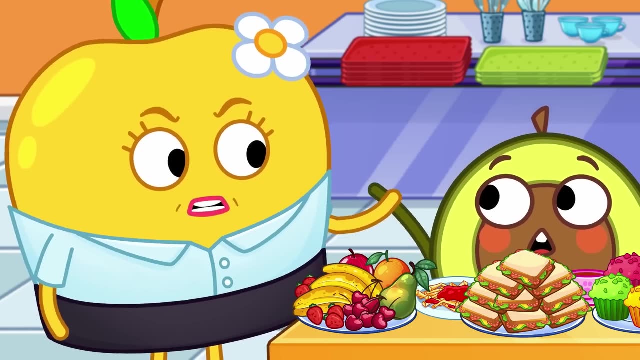 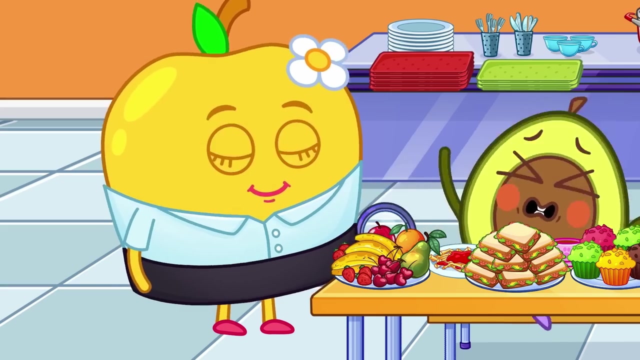 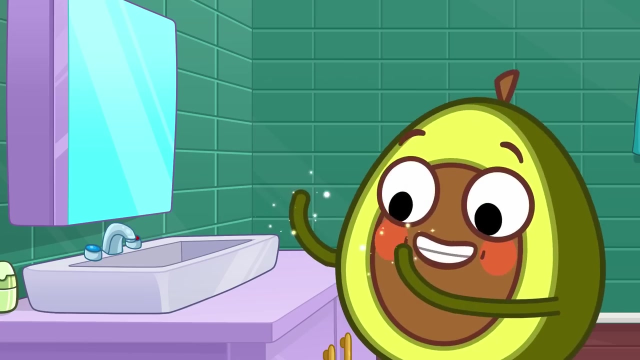 It's for a special lesson. Today we will learn table manners. Wait, Pit, You haven't washed your hands. They're dirty and covered in germs. Soap and water gets them nice and clean And we can use them for the night. 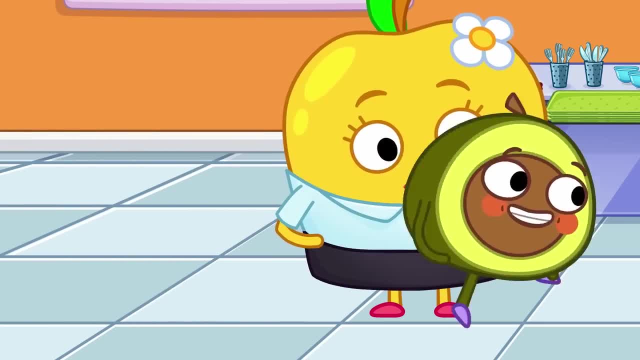 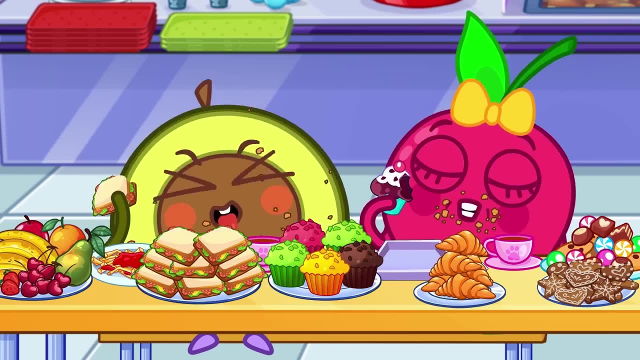 We have to go上 and back. Goodbye Pit. The table is gone and our house is gone. Too late, Perry. We can do nothing but fool around. The table is empty and I have to go to sleep. I can't do anything. 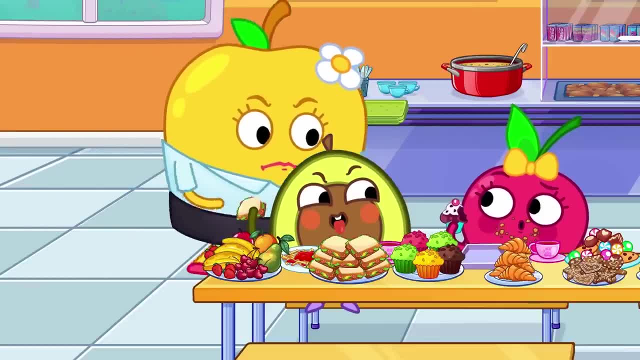 I have to go to bed. I think I'll go to sleep. I'm going to bed too. No, you can't. They won't let me. You will go to bed with me. I can't, ног. I'm going to bed. 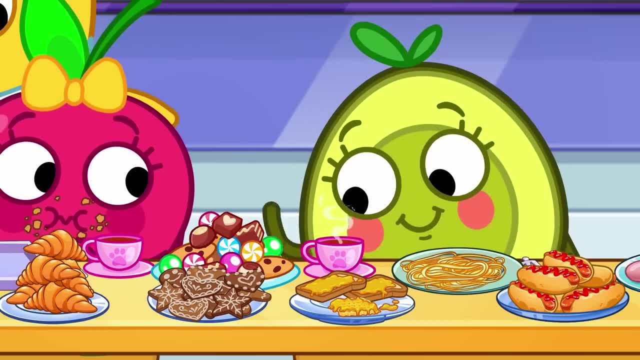 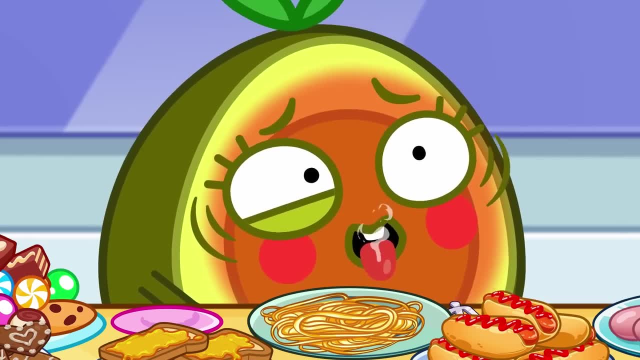 You can't. I'm going to bed. I'm going to bed. I'm going to bed. You're lying Me, Me. You won't be able to go Me. You won't be able to go to bed. Penny's tea is too hot. 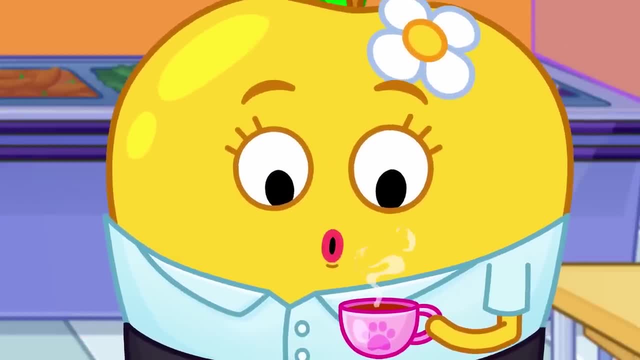 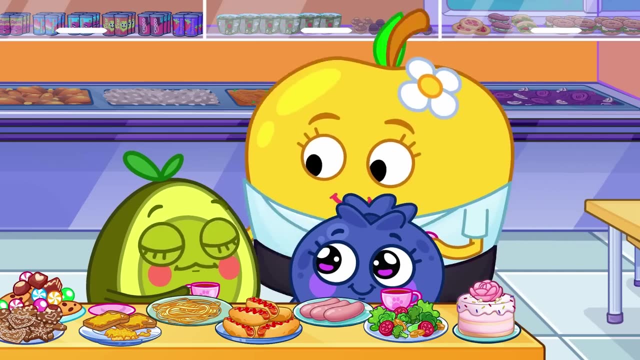 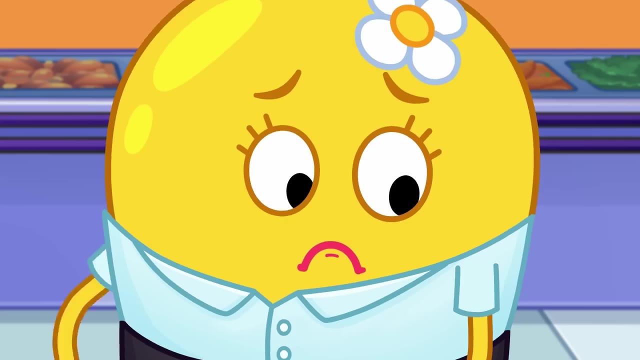 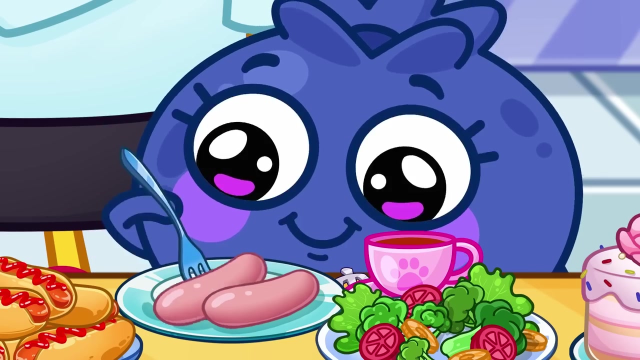 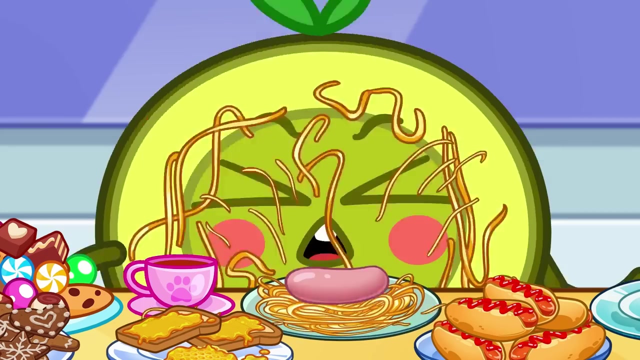 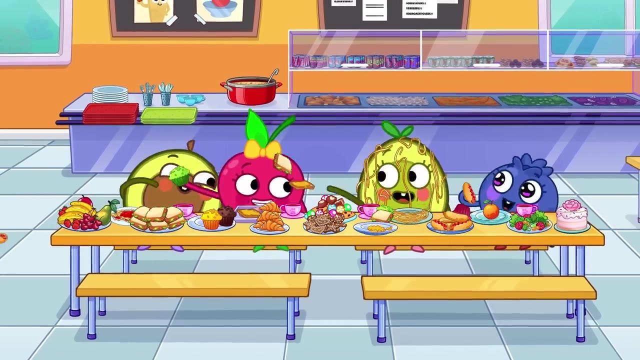 Drink hot tea carefully. Blow on it first to cool it down. Now it's safe to drink. Blueberry is eating with his hands. Oh, use your fork please, Poor Penny. No, kids, don't play with your food. 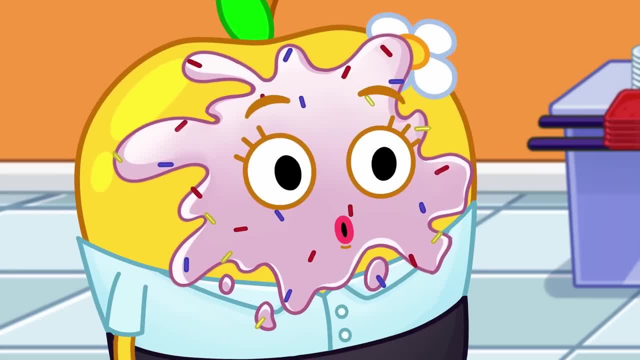 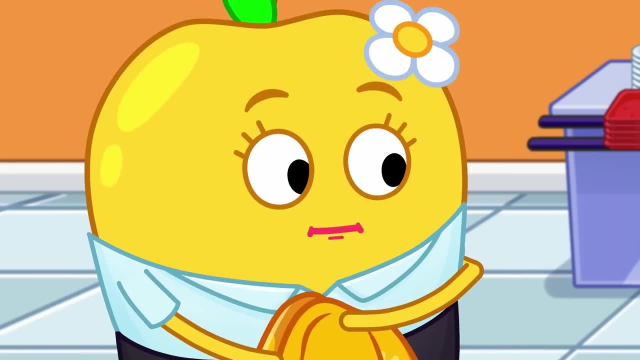 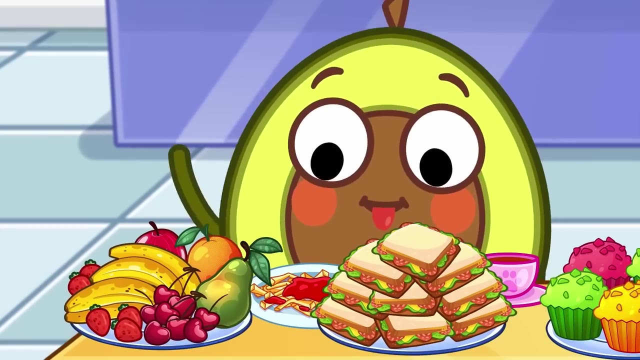 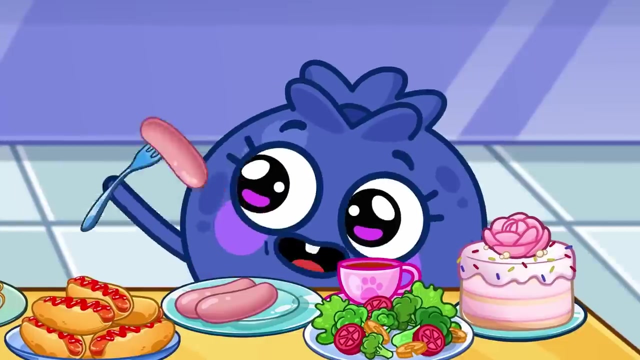 Look what you did to Miss Apple. Oh, We're sorry, You can't play food at the table. Remember to wash your hands. Eat with your mouth closed, cool your hot tea and eat with a fork. Good job, kids. 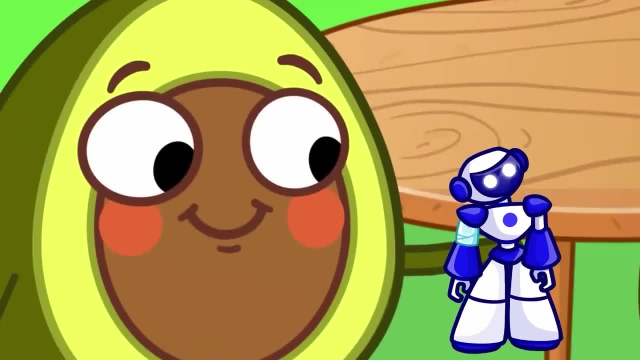 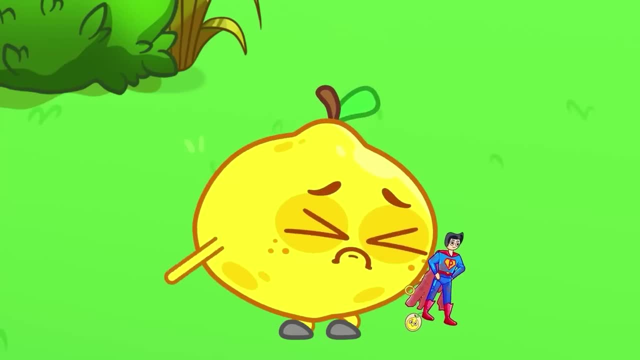 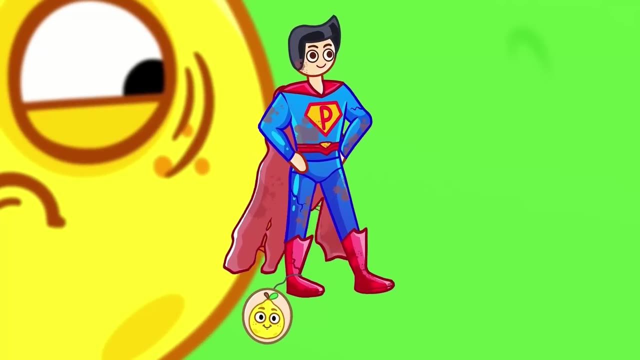 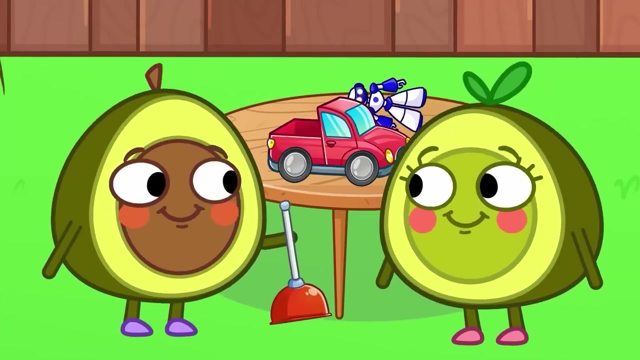 Very good And Penny fixed the toy robot. I will save you. Now. it's as good as new. What's wrong? little lemon, I am super. Oh, his toy is broken. Pete and Penny have fixed all their toys. I have no toys. 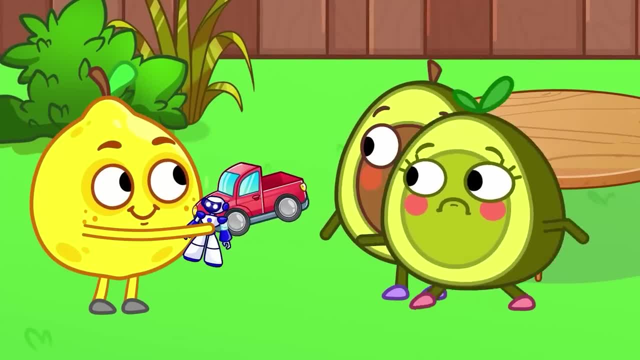 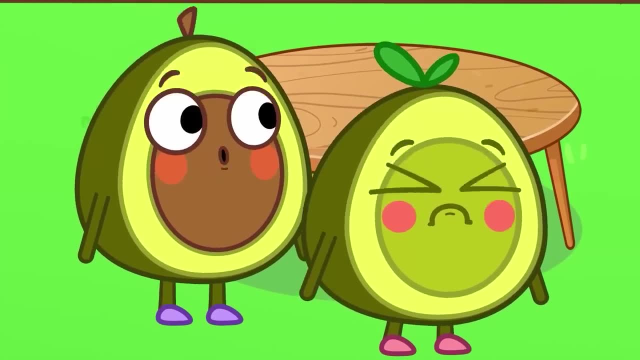 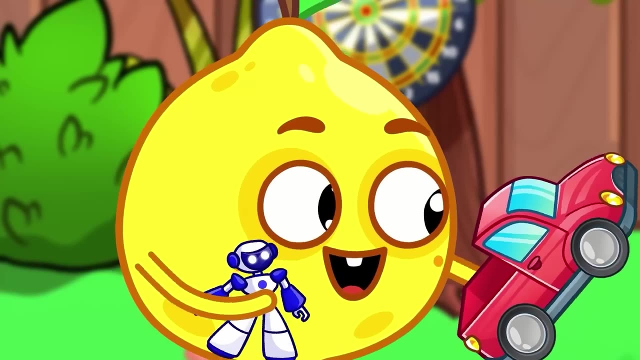 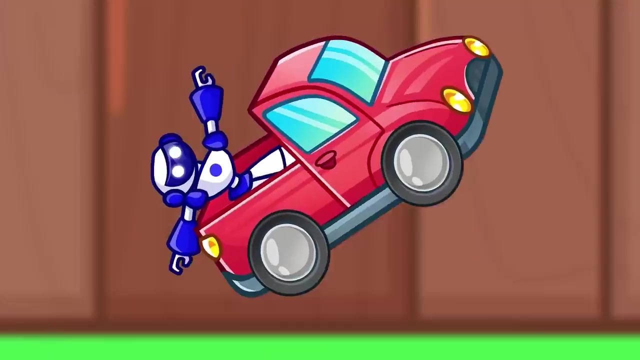 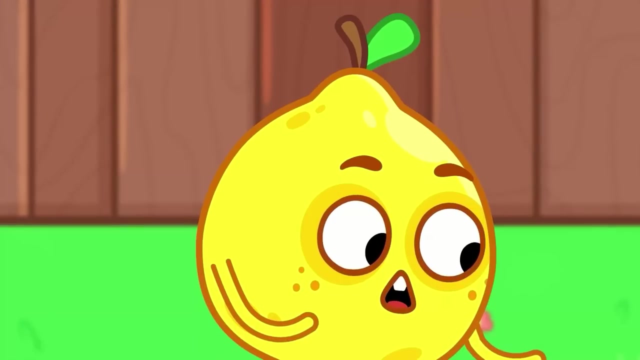 Oh, You can play with Pete and Penny's things. Oh Wow, It's a stoned car track. Oh no, You've broken the toys. I can't see what you've done. little lemon, Ugh, How many times do you want to get hit? 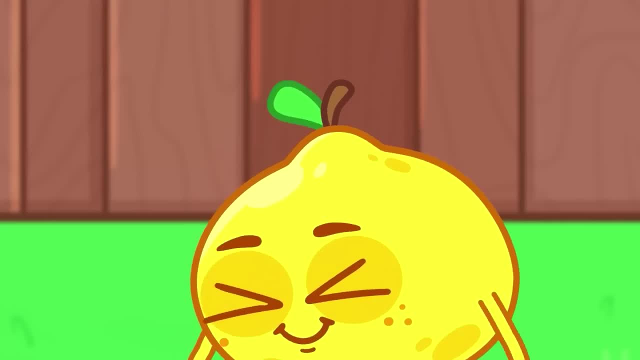 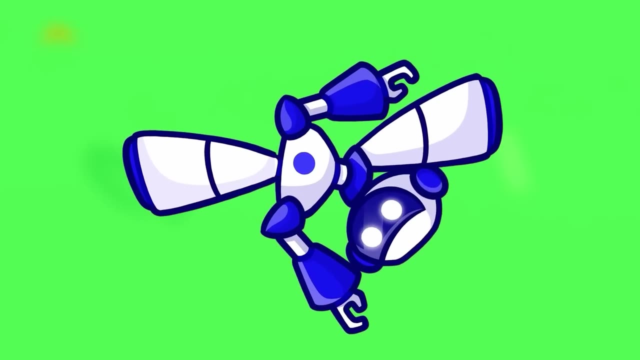 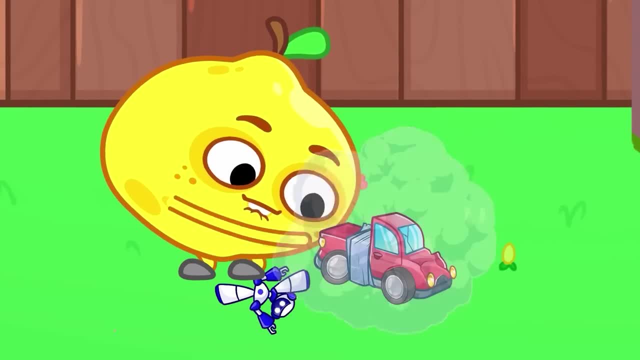 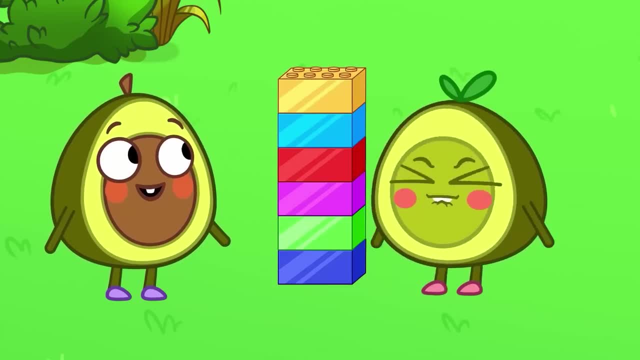 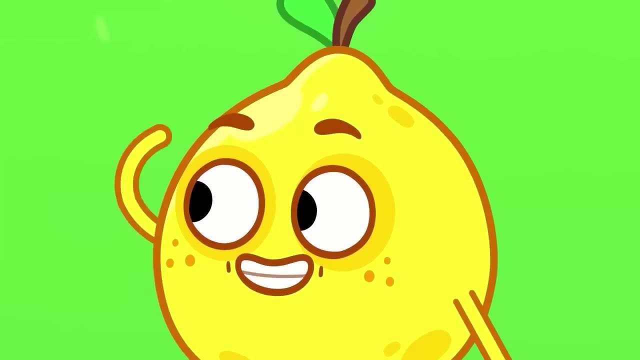 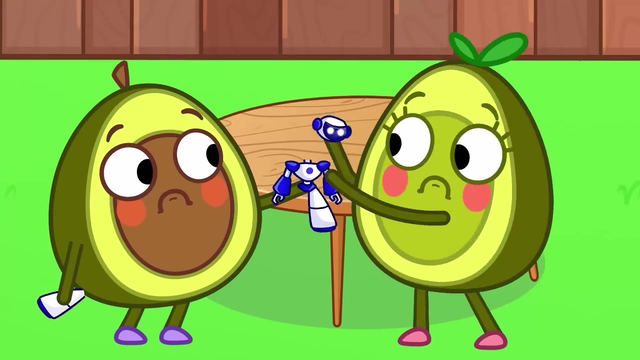 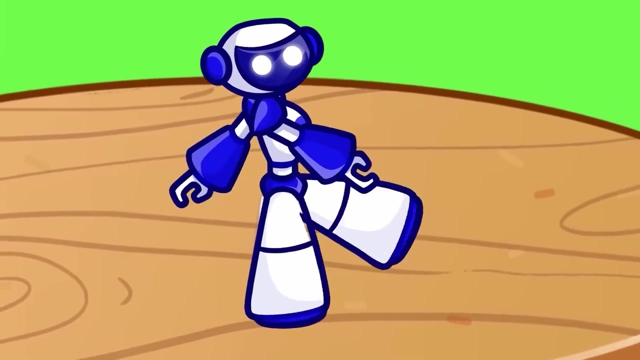 That's too much. No, no, no, no, Don't kill me, Don't you hear me? Ah, A little lemon brought your toys back And they are still broken. Pit fixed the robot. Can I play with the robot? 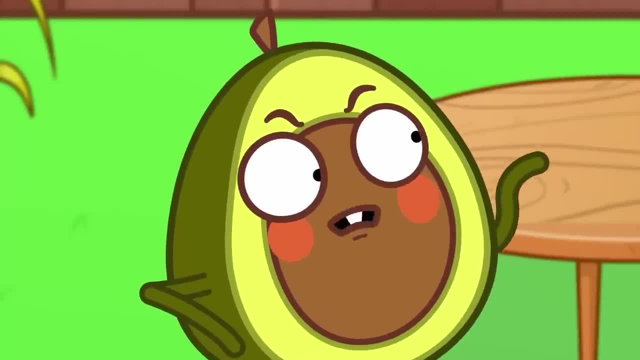 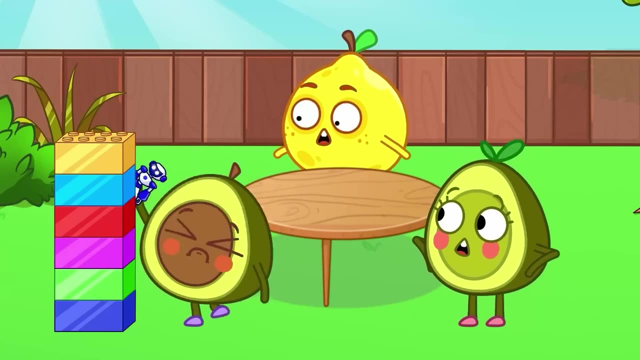 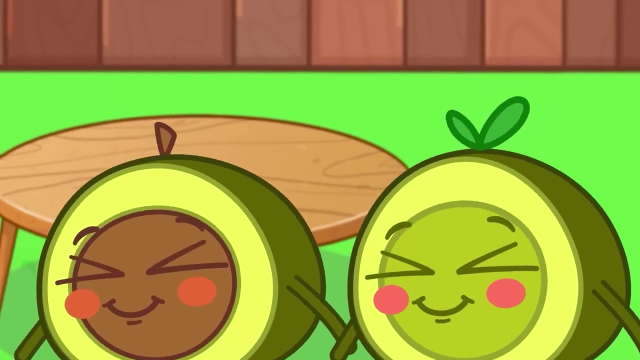 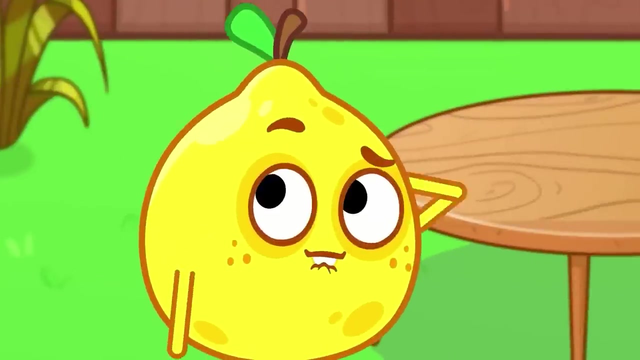 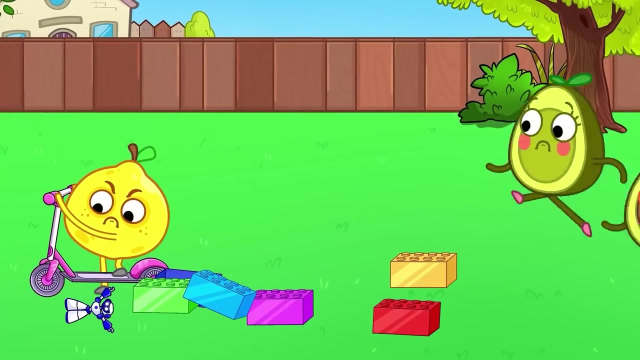 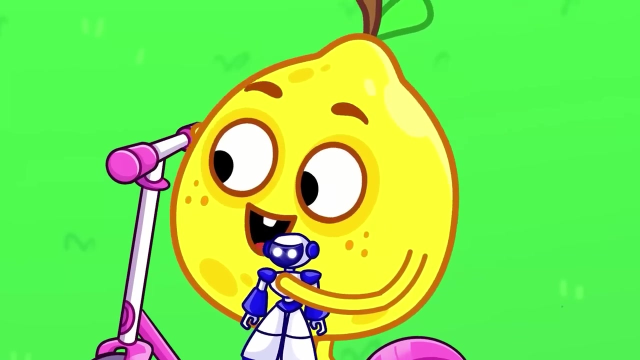 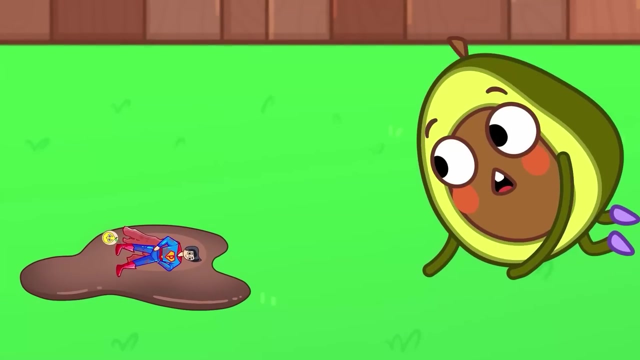 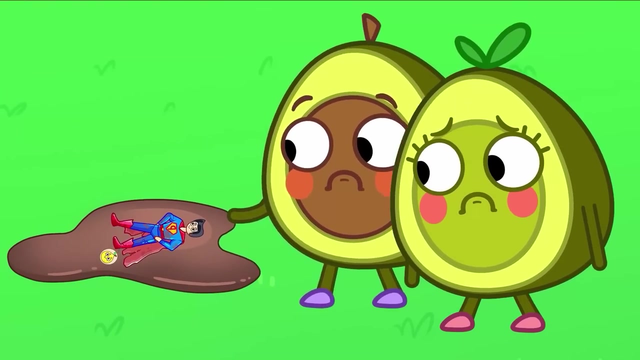 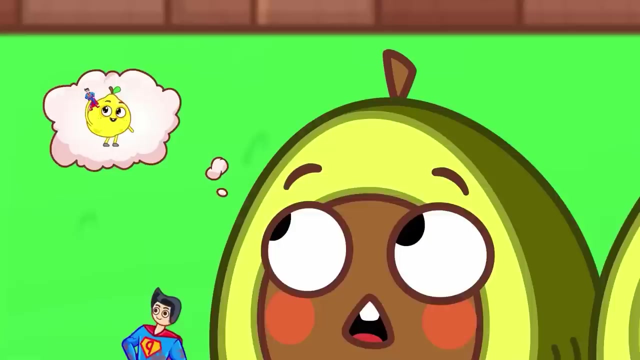 Why not Pit? You don't know how to play with toys. You need to be more careful, little lemon. Little lemon has a plan. Now he has the toy robot. That was little lemon's favorite toy. The kids have a plan. 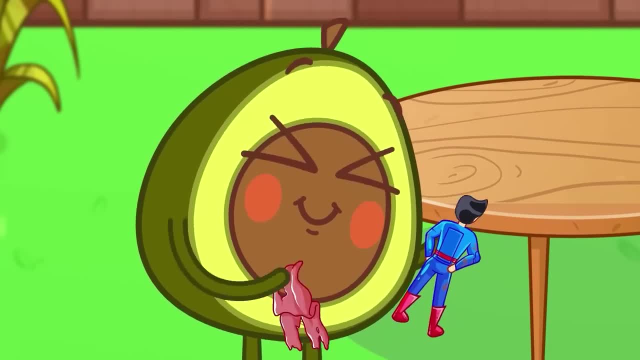 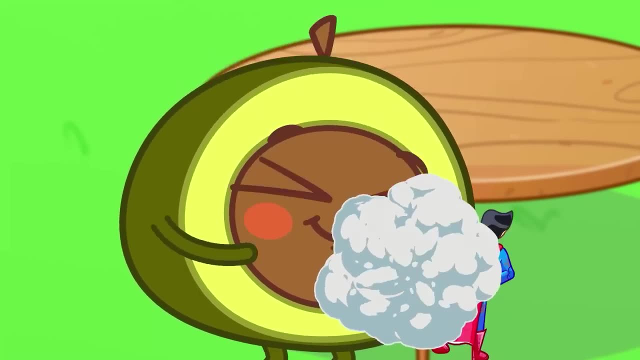 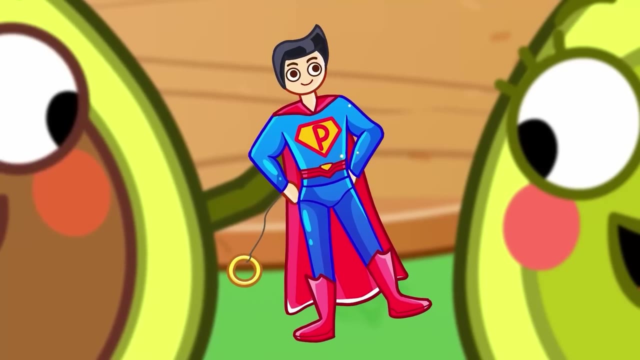 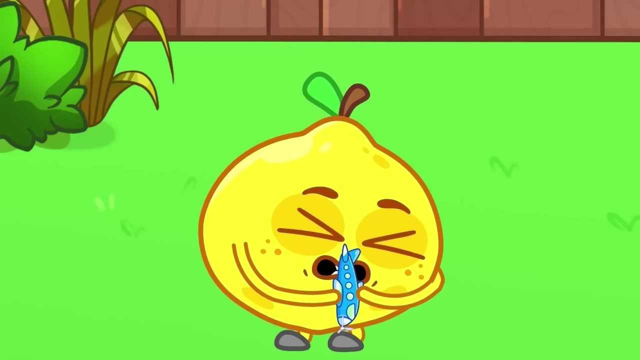 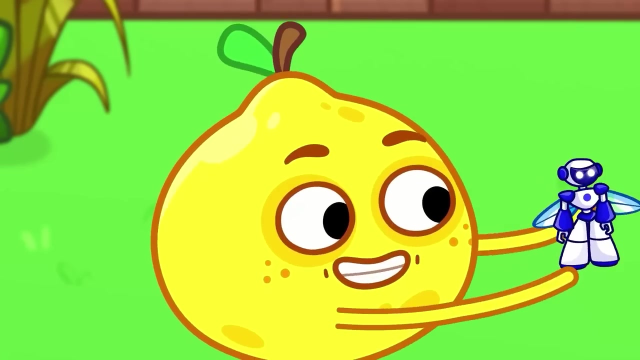 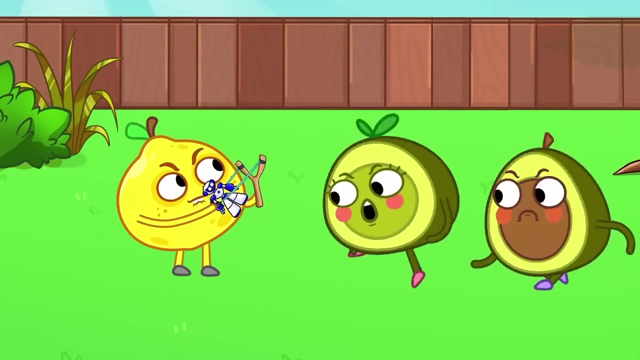 They'll add a new battery, Make a new cape And clean the towel. I am Superman. Hey, little lemon, You need to clean your house And clean the room. Be careful, I got you. You're cute. I love you, little lemon. 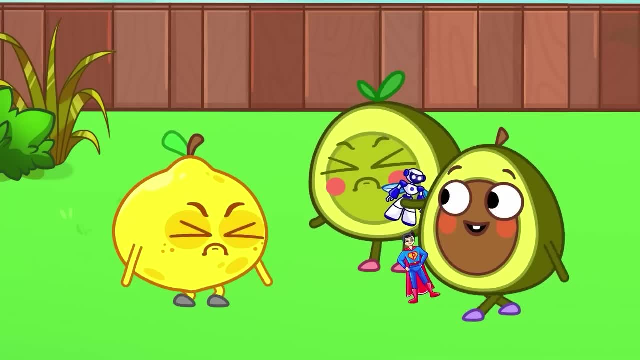 Ow, It hurts. Even if I get hurt, I will never do this again. Hey, little lemon Youuri, you're too big, You're just too tall. Be careful with the toy robot. We don't want to hurt you. 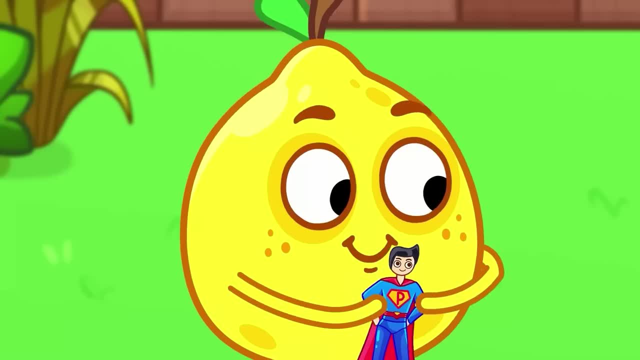 So I brought them back. What little lemon is doing? What little lemon is doing? Don't do that. Wouldn't you rather play with this doll? Play with your toys carefully, that will be like new. I am sorry, I will take care of my toys. 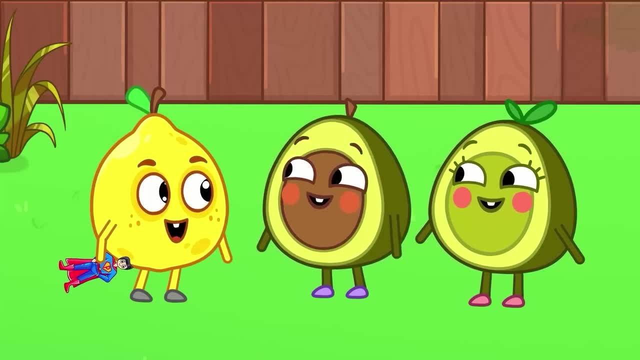 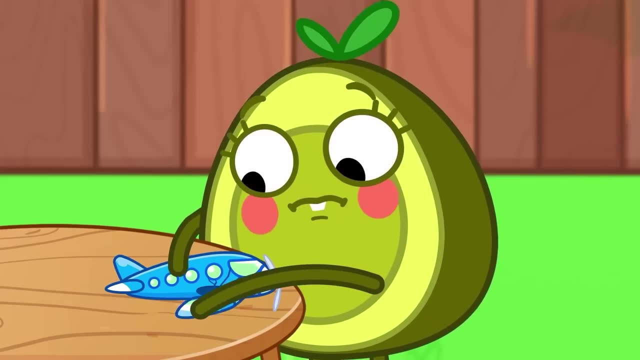 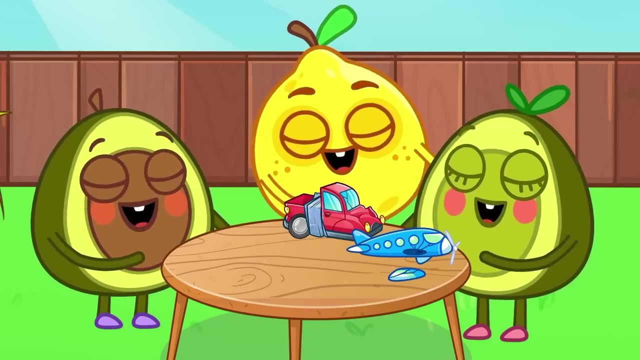 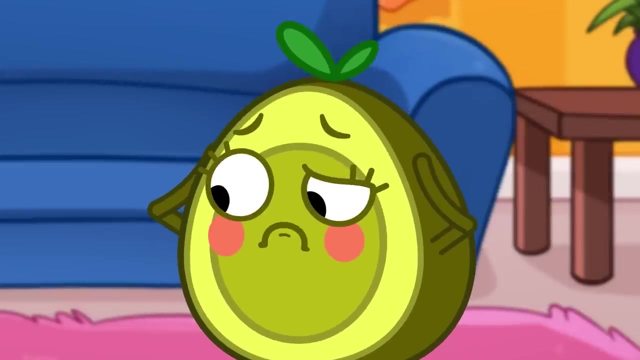 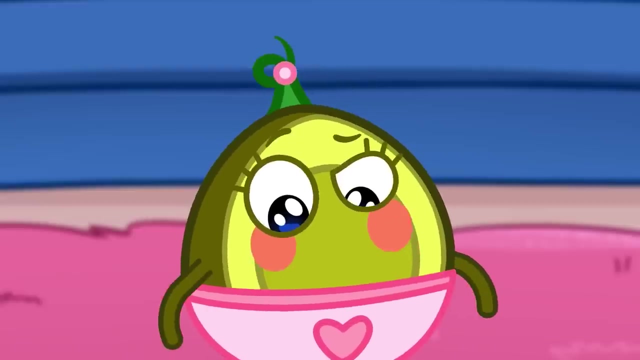 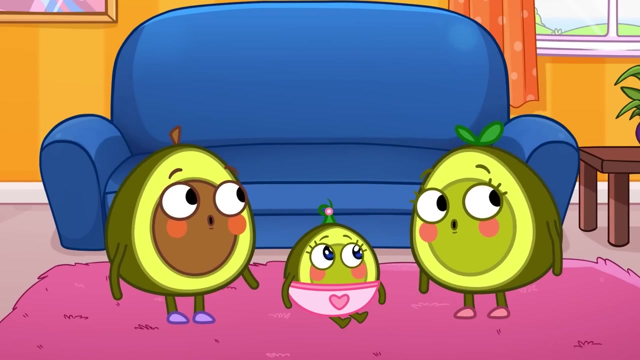 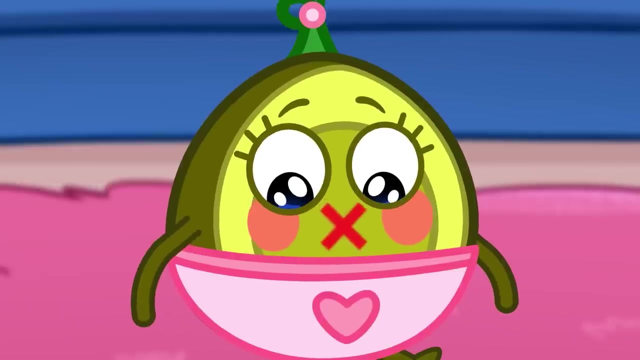 my toys. Let's fix the broken toys first. Keep trying, little lemon. Oh no, Baby's crying. Why are babies so loud There? Baby stopped crying, But her mouth is missing. Where did it go? It's time to feed your little sister, But she can't eat without a mouth. 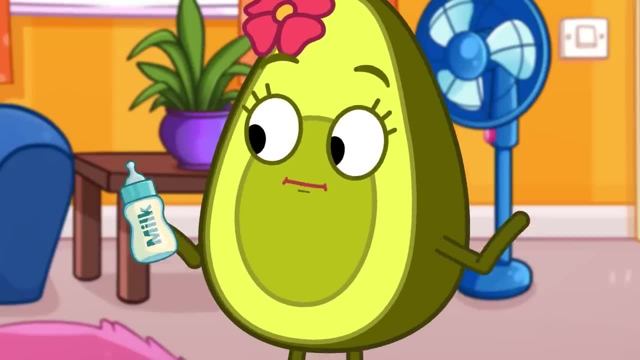 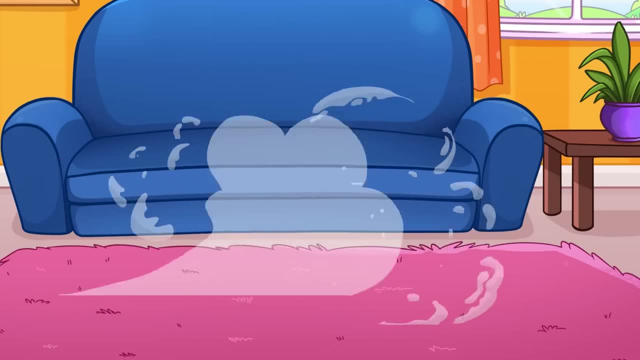 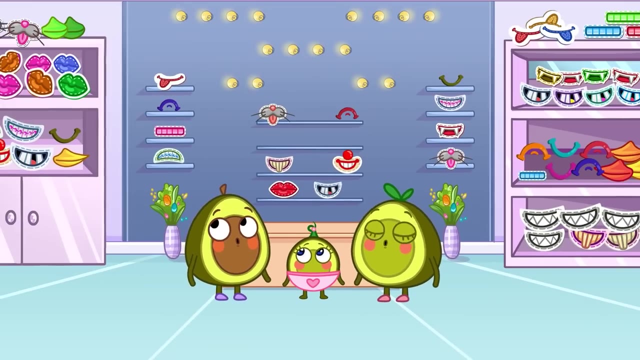 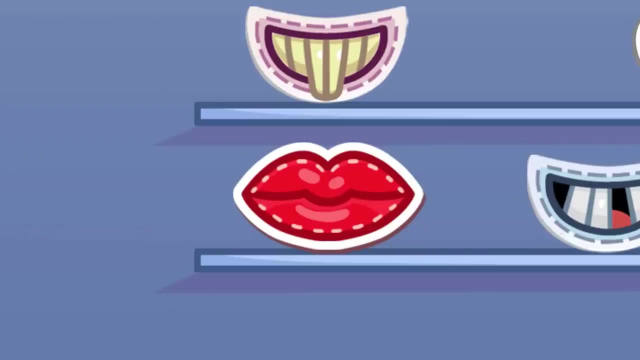 We will feed you. We will feed her. You'll need to find her mouth first. Let's check out the mouth store. Look at all the mouths. We need to find a new mouth. There's a pair of kissy lips, But they might not be right for her. 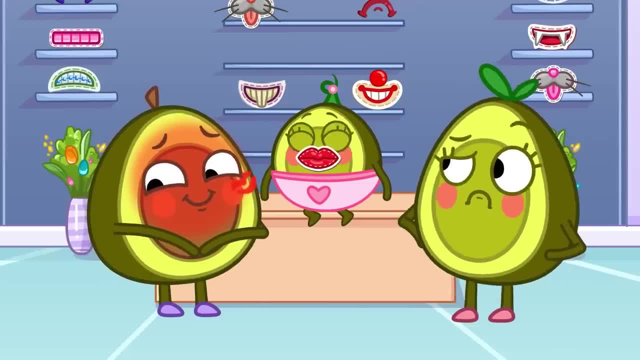 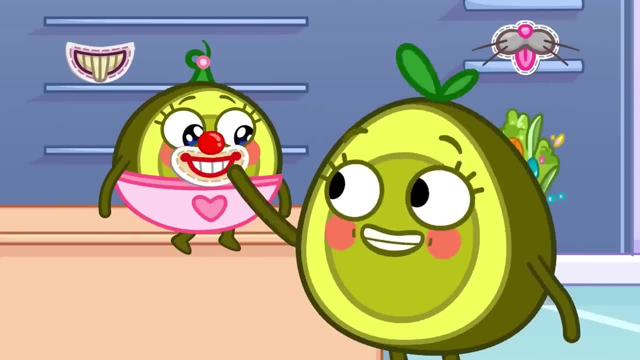 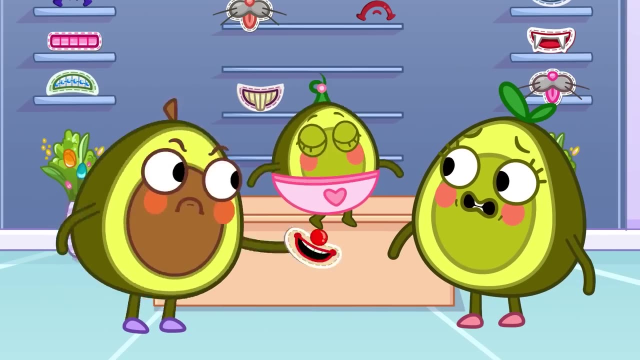 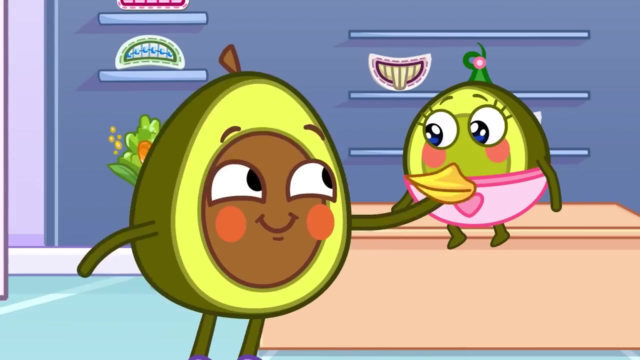 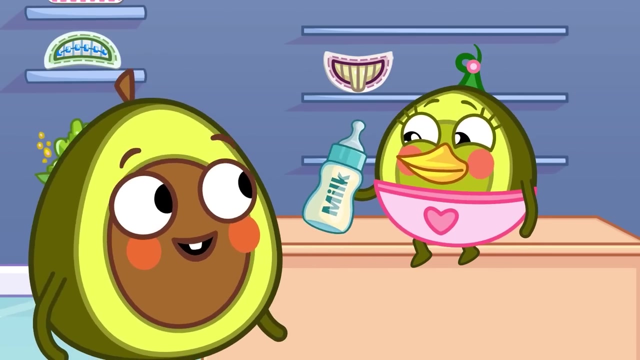 They might not be right for Baby. That one has a clown nose. But Baby's not a clown. Oh Pit, That's a bird's beak. Baby picked holes in the bottle. Baby picked holes in the bottle. Baby picked holes in the bottle. 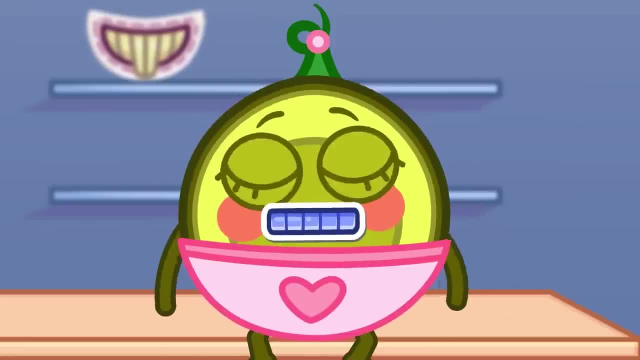 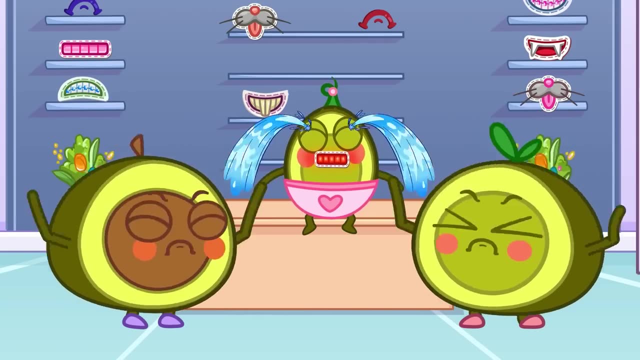 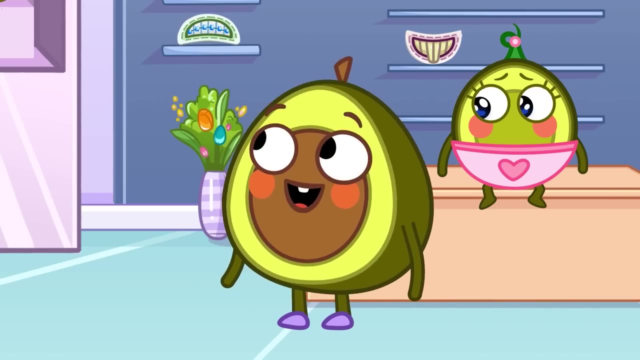 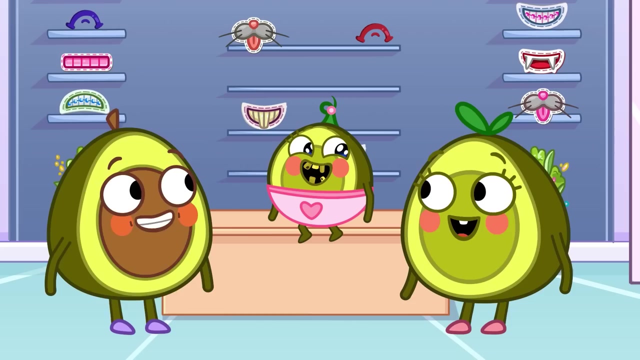 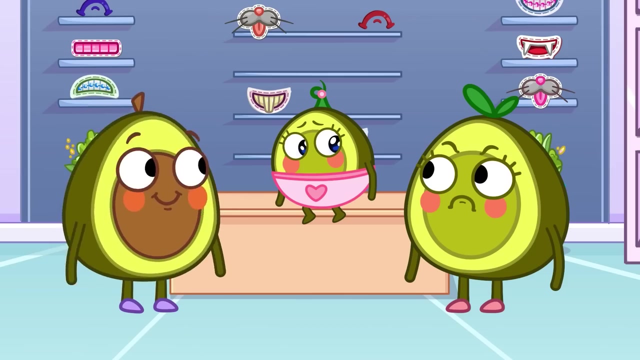 Penny, that's a robot mouth. Penny, that's a robot mouth. You'll have to keep looking. You'll have to keep looking. That smiley mouth looks good. It's filled with stinky Qi. Maybe Baby can pick her own mouth. 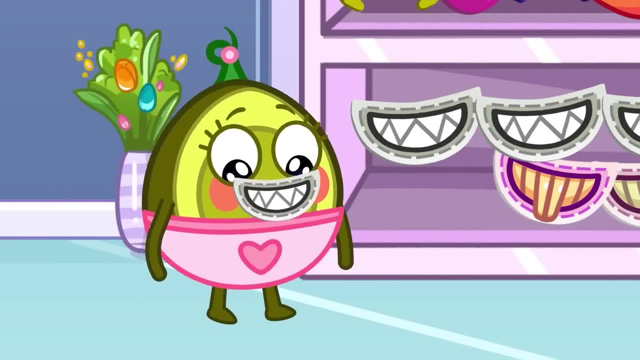 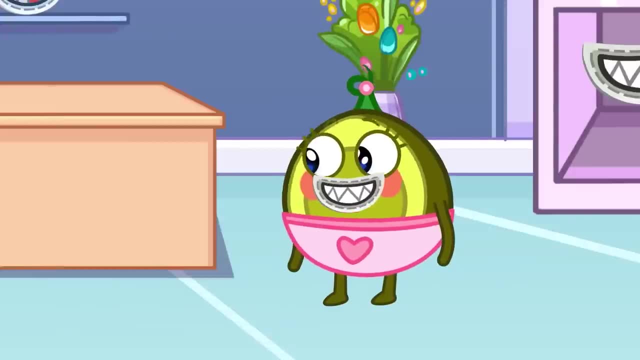 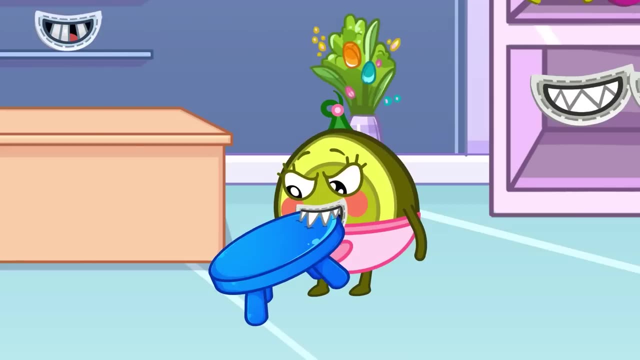 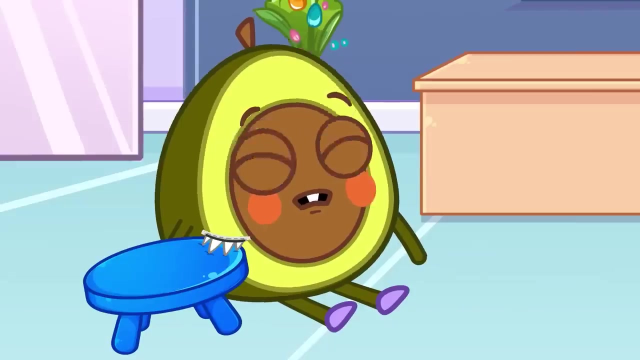 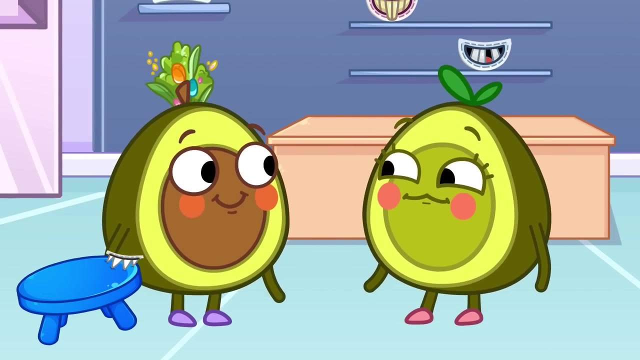 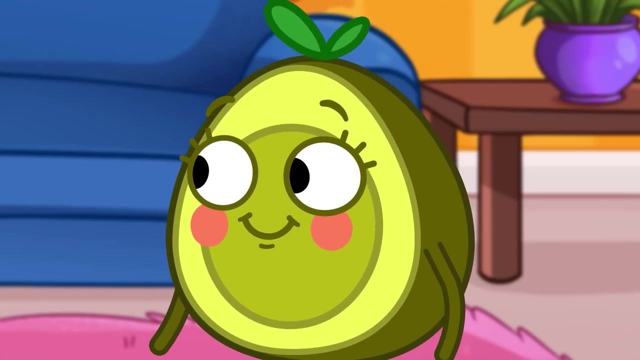 But those have very sharp teeth, os theseอะไร Please, no, Please, no, Don't get too close kids. Now what will Pit and Penny do? Phew, It was just a daydream. Baby can drink from her bottle. 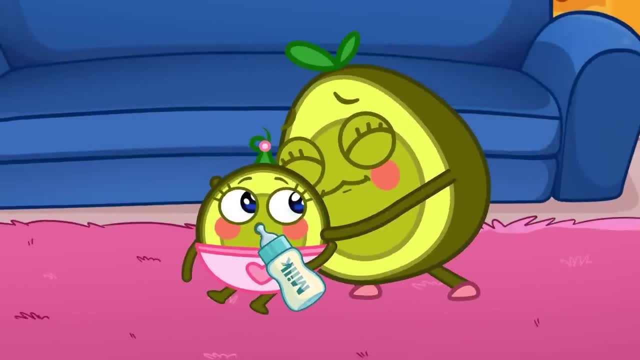 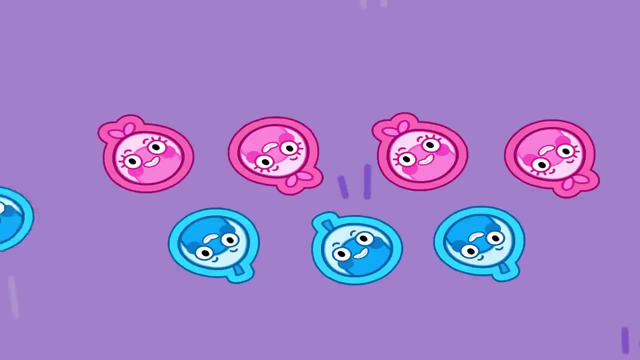 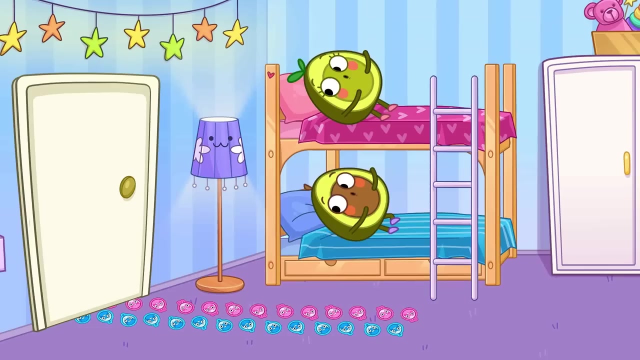 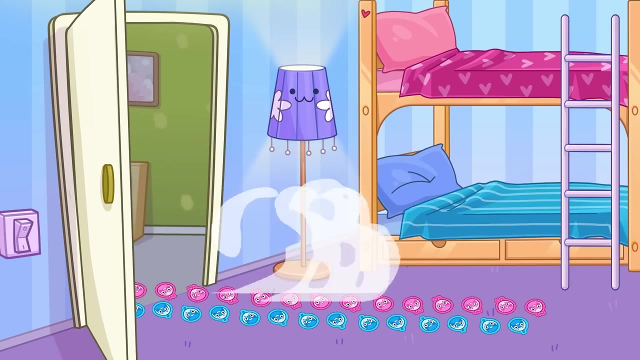 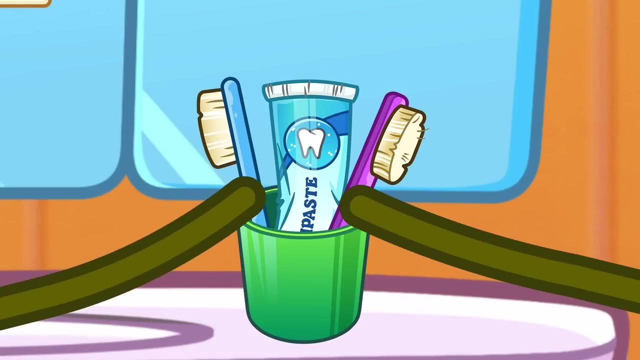 I'm so glad she has a mouth And she has stopped crying. Mommy and Daddy have a surprise for the kids. Wake up Pit and Penny. Follow the stickers to the first challenge. Let's start by brushing your teeth. Brushing keeps your teeth healthy. 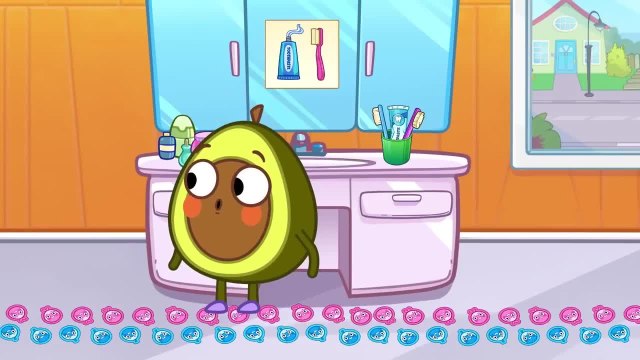 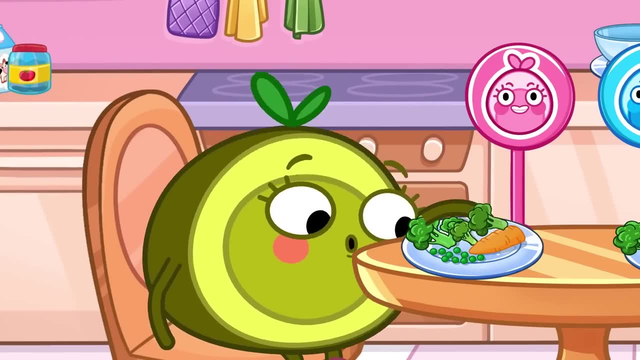 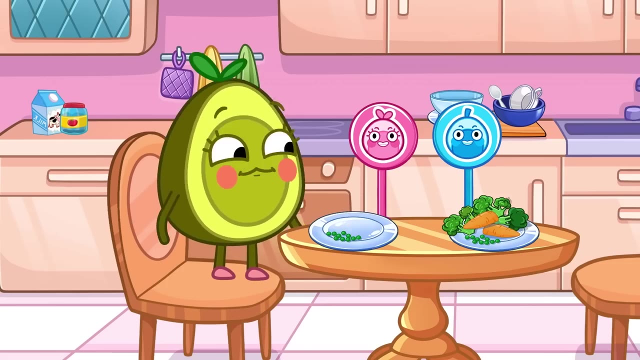 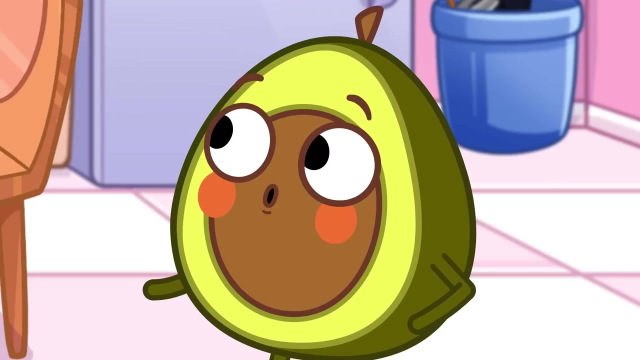 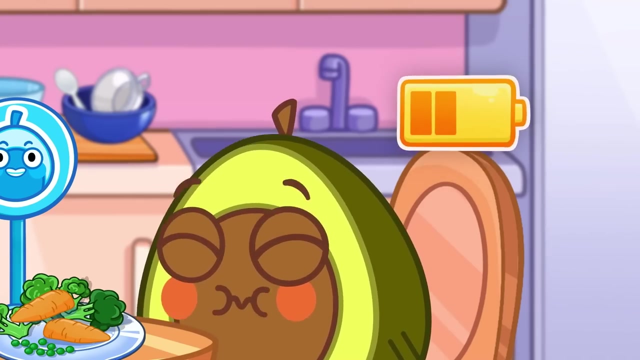 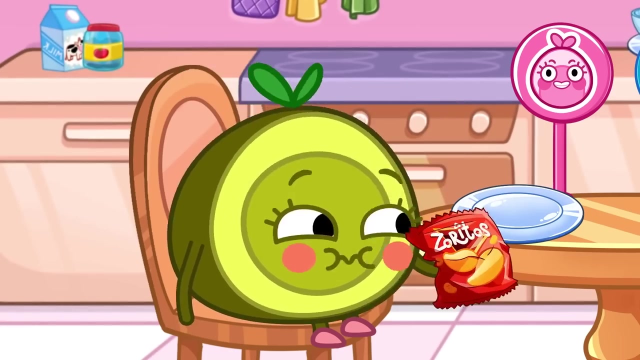 Penny doesn't want to brush. Penny doesn't want to brush. Next challenge: eat your vegetables, Penny. that's cheating, Cheating. Vegetables give you lots of energy. Vegetables give you lots of energy, But junk food doesn't. 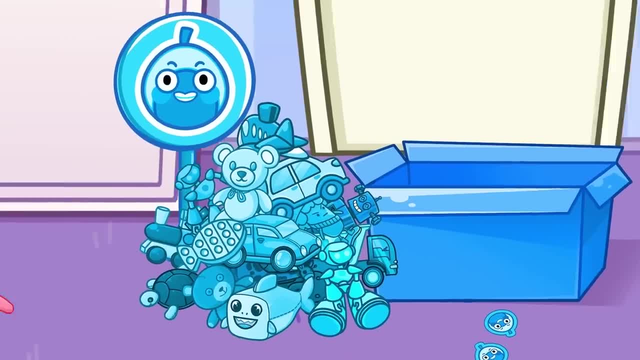 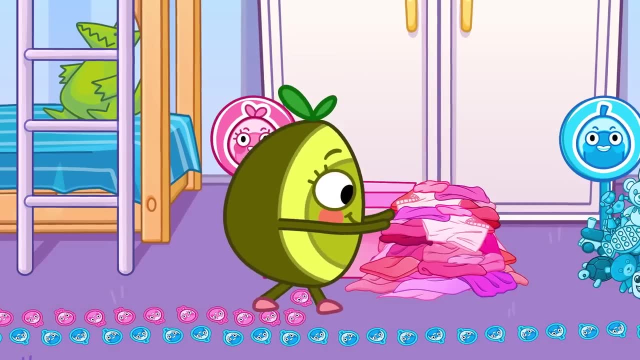 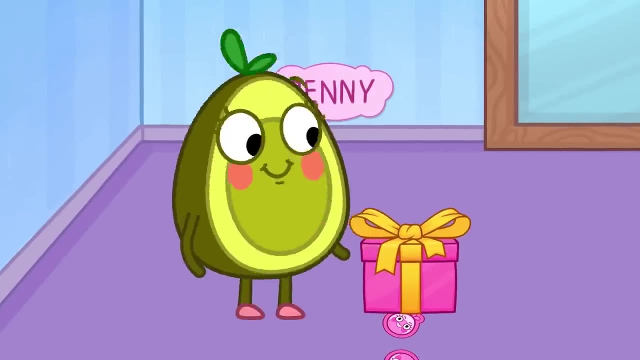 Now you have to sort your things, Penny. But Penny's too tired to work. She'll make Pit sort through everything. She'll make Pit sort through everything. She'll make Pit sort through everything. Make a castle out of stickers, Penny. 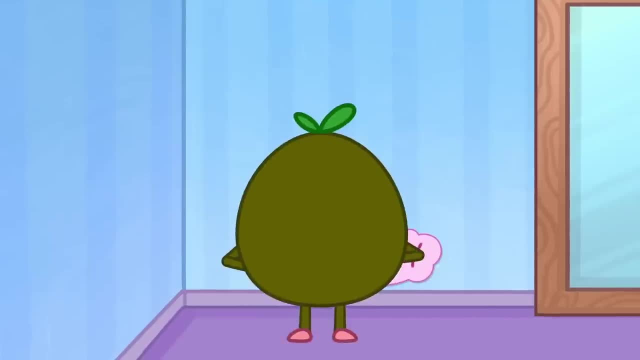 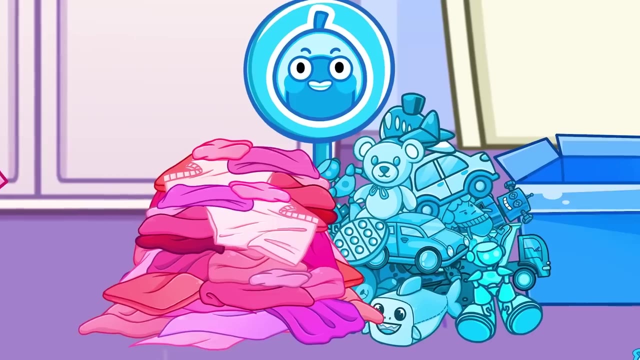 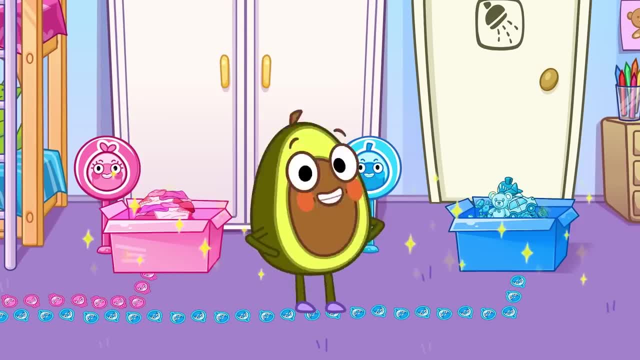 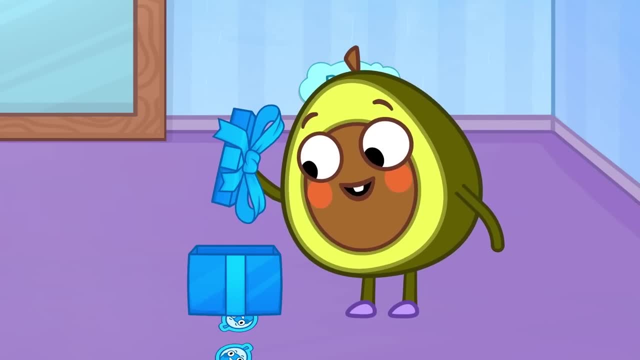 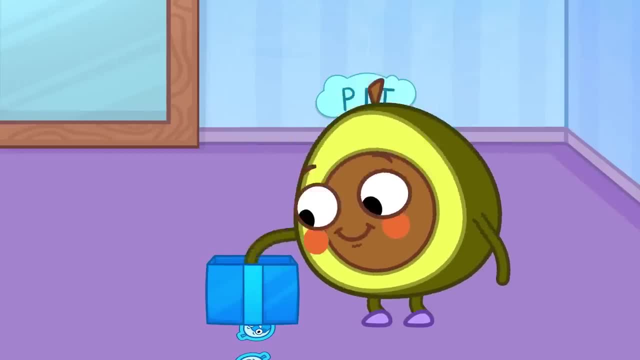 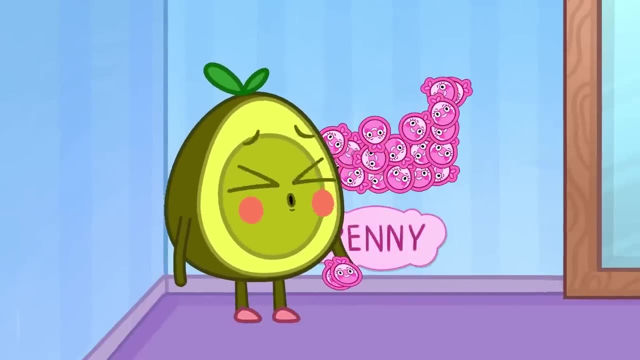 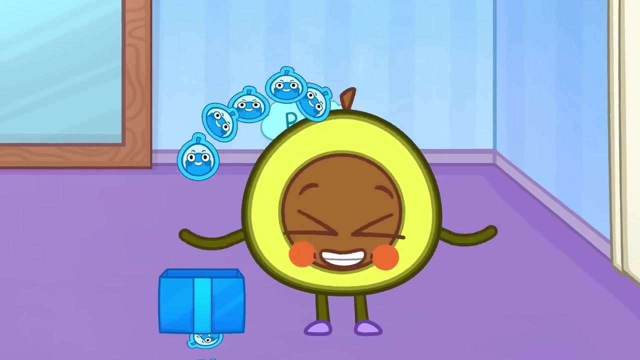 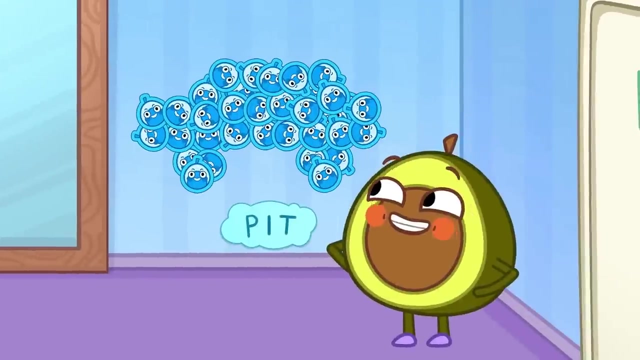 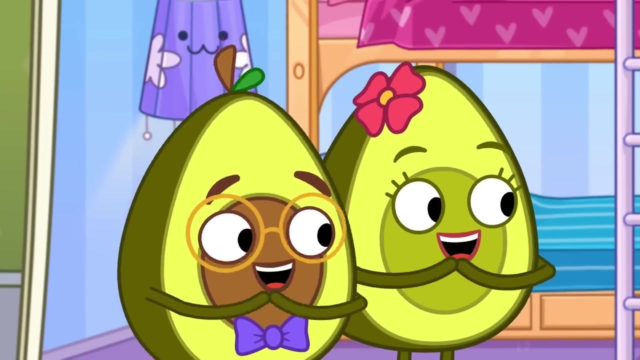 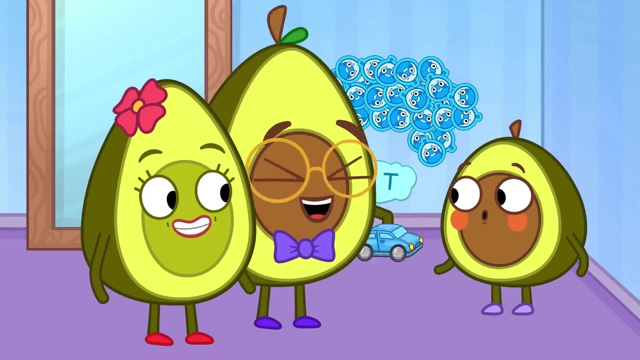 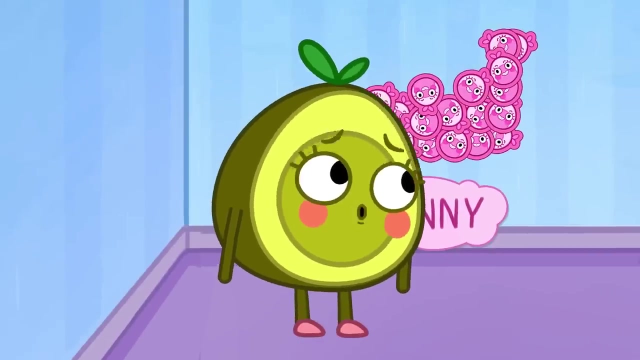 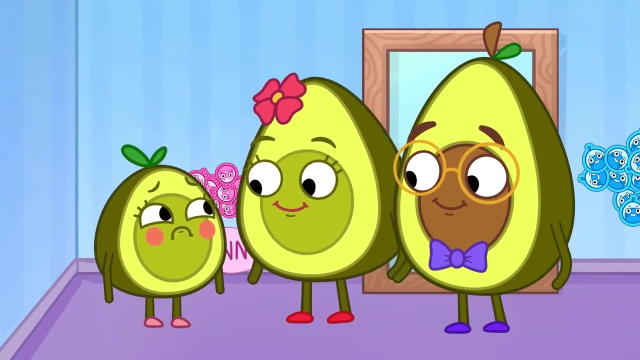 Penny has no energy left. Pit has lots of energy. Pit finished all the challenges first. You have won Pit. Your prize is a toy car. I won a prize too, Darn it. You need to be hardworking Like Pit was today. 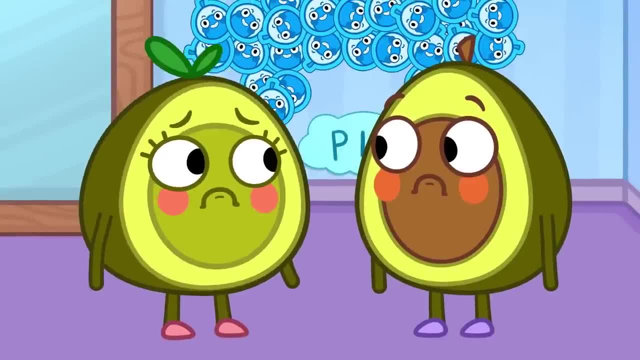 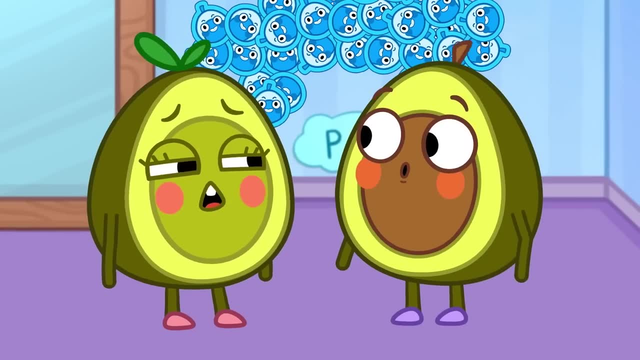 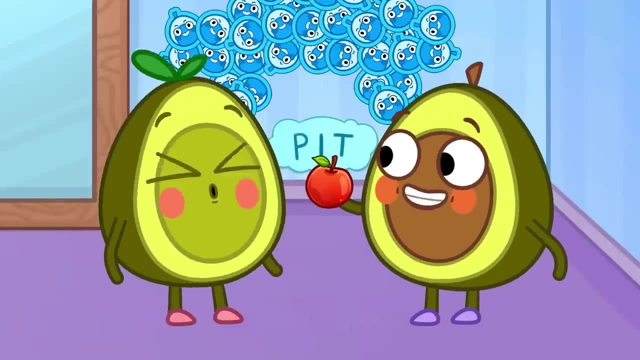 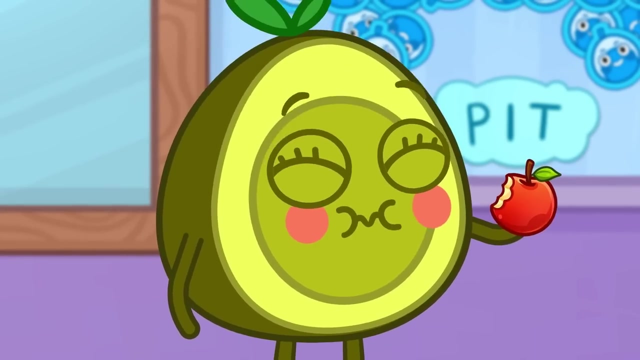 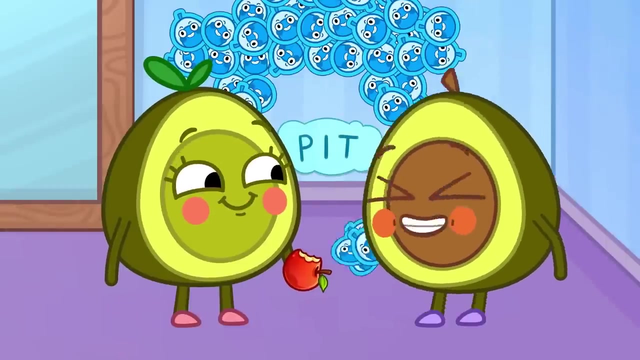 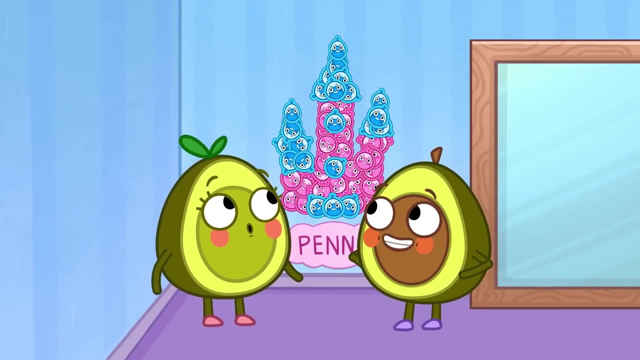 I'm sorry, I'll be hardworking too. Pit knows how to help Penny To be hardworking. you need to eat well, And fruit gives you lots of energy. I will help you. Yay, Now, Penny gets a prize. 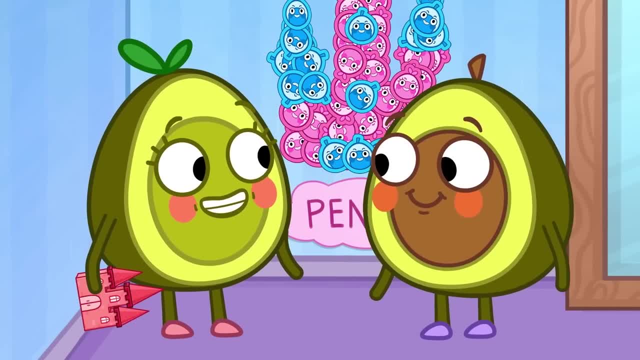 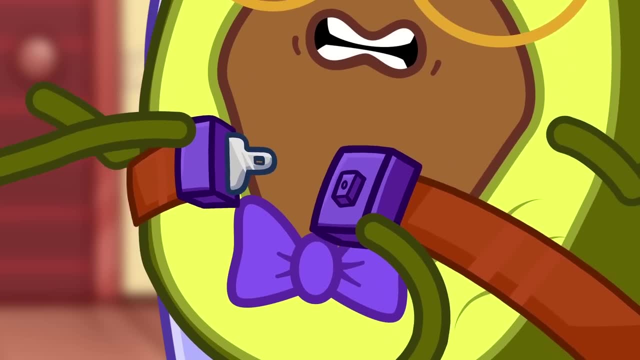 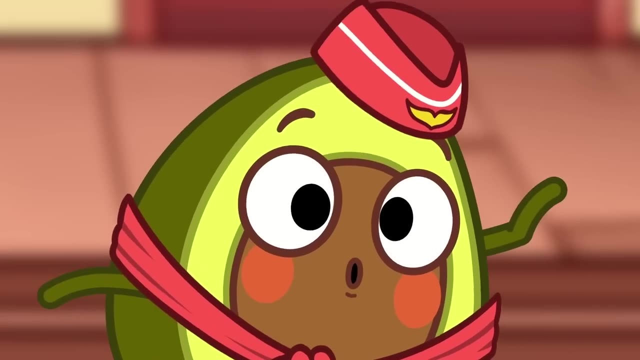 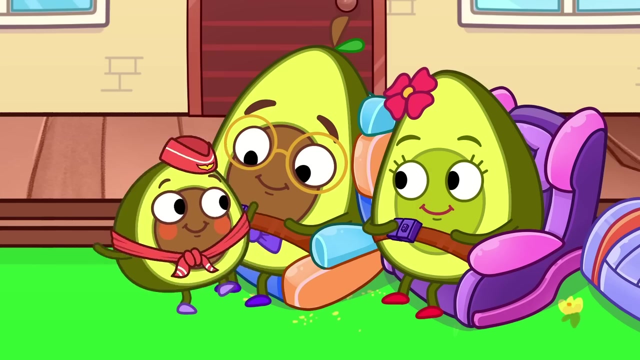 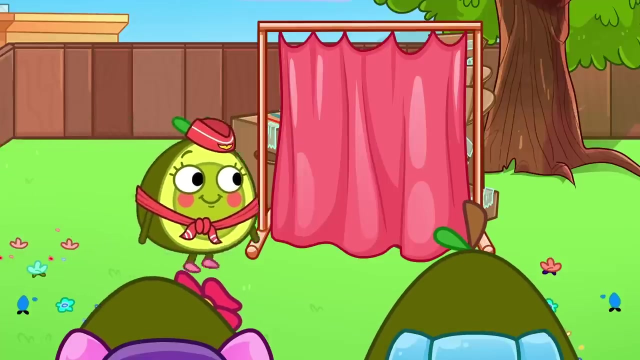 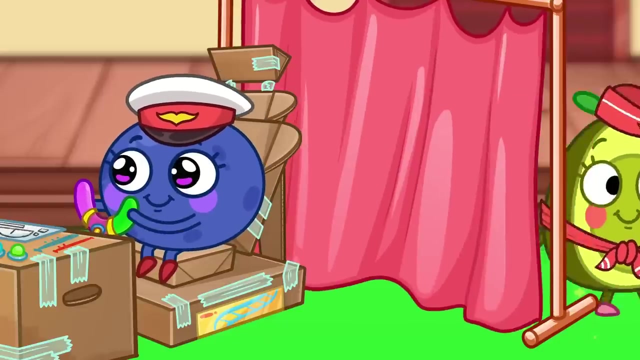 Great job, kids Pilot. Blueberry is ready to take off, But first the passengers must put on their seatbelts. Daddy's belt is. It's a little tight. You did it. Pit Your turn, Mommy. Everyone's ready, Blueberry. 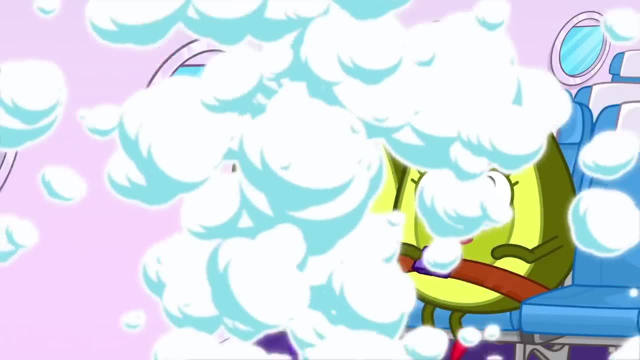 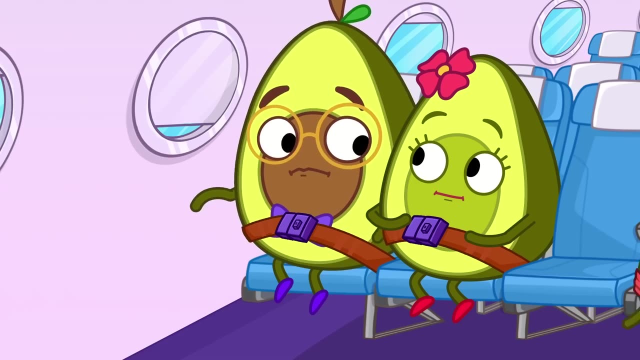 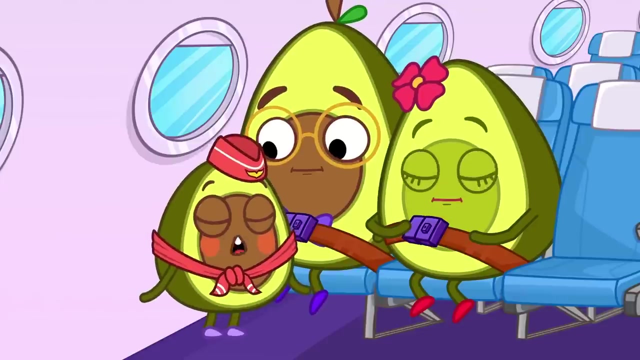 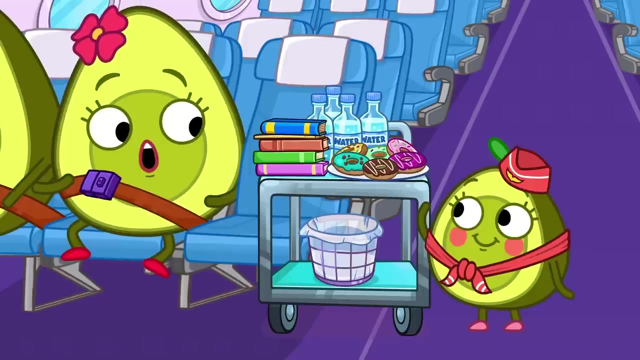 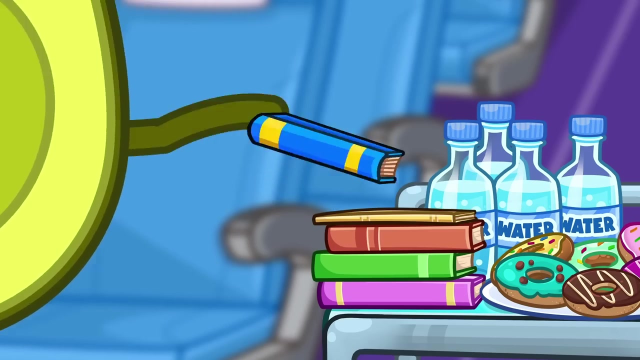 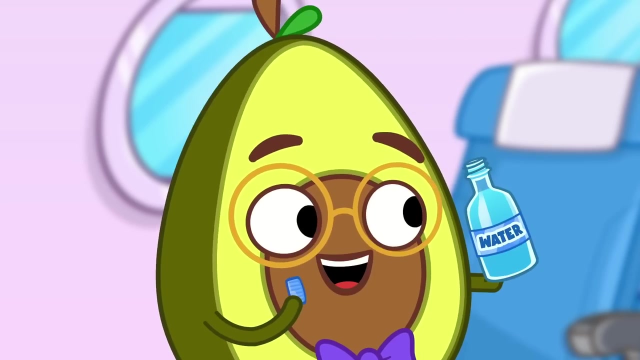 The sun is in Daddy's eyes. The window blinds must be open during takeoff and landing. Does Mommy want something from the cart? What Mommy wants to read? And would Daddy like something from the cart? He chose a bottle of water. 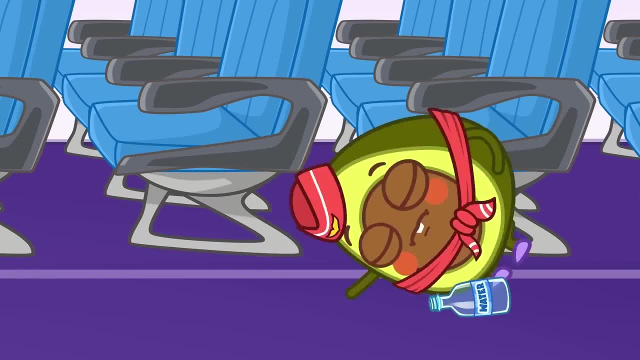 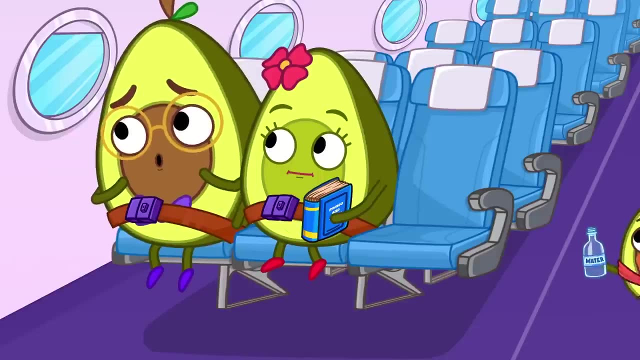 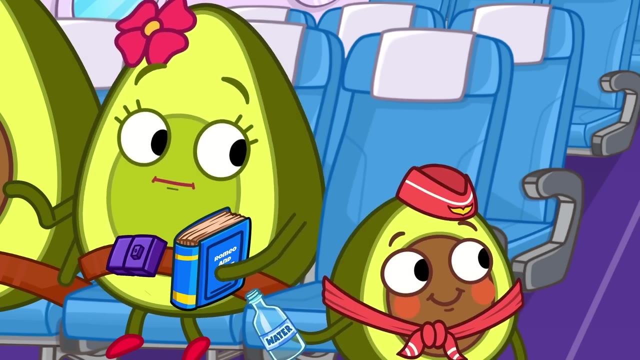 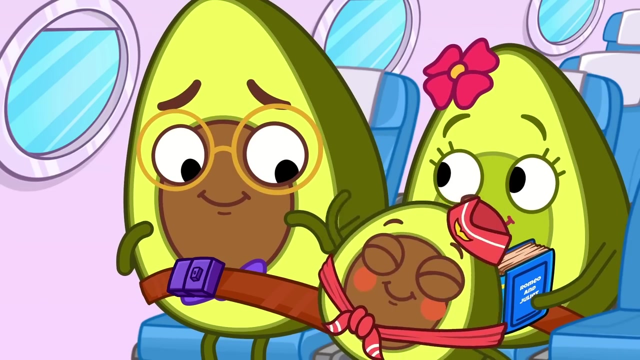 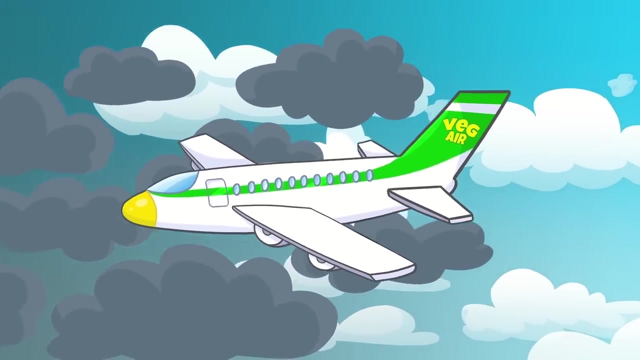 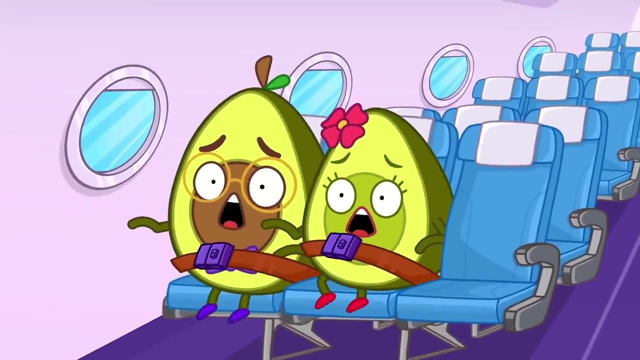 Watch out, Pit. You need to tell Daddy the rules. Oh, Throw your trash in the bed. Do you understand, Daddy? Hehehe, What's going on? Mommy and Daddy don't need to worry, Don't be afraid. 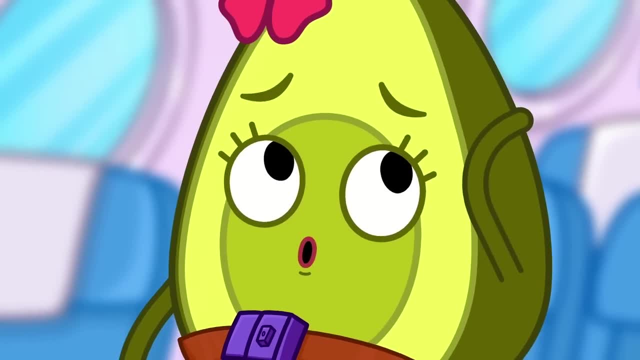 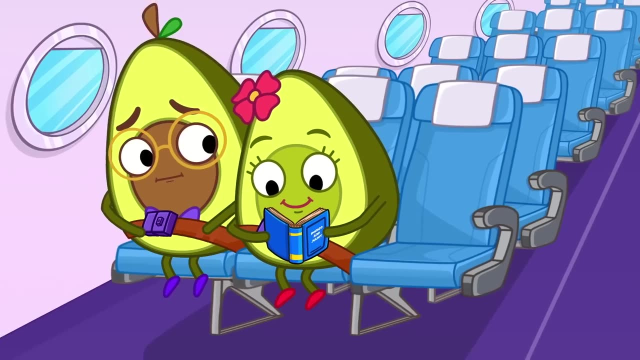 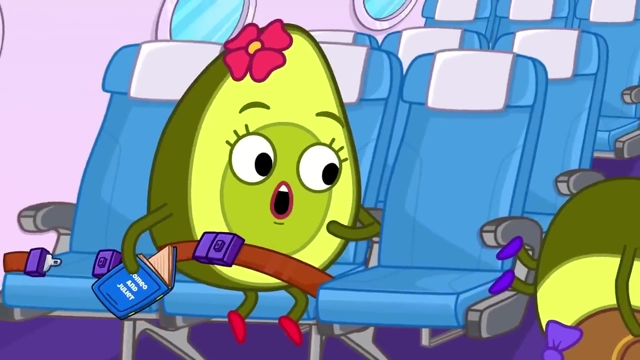 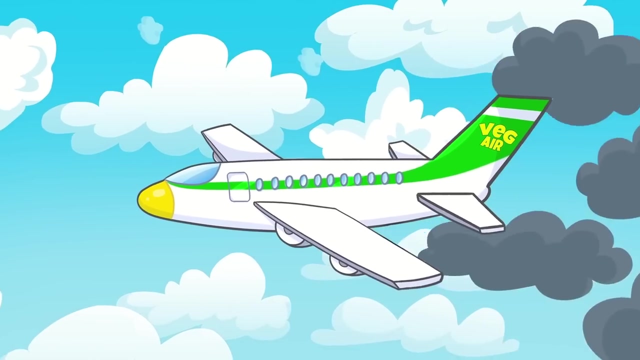 It's just some turbulence Now. Daddy needs to use the restroom. But Daddy should wait in his seat. You're in turbulence. You need to stay in your seat. It's now safe to use the restroom. It's now safe to use the restroom. 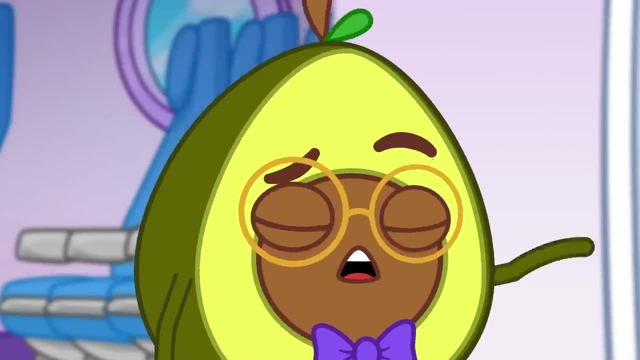 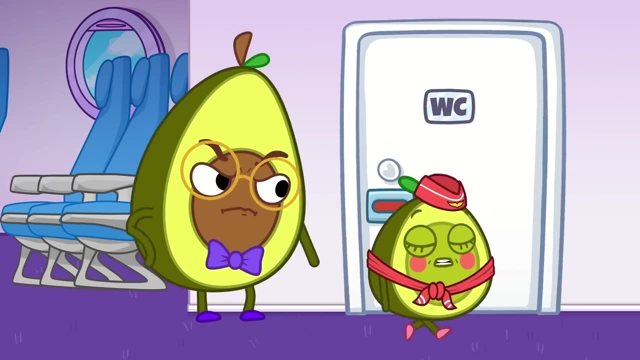 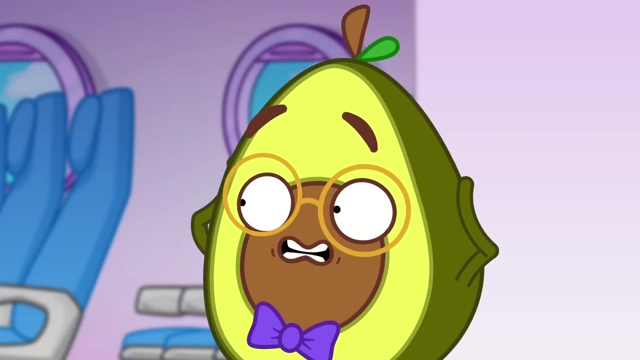 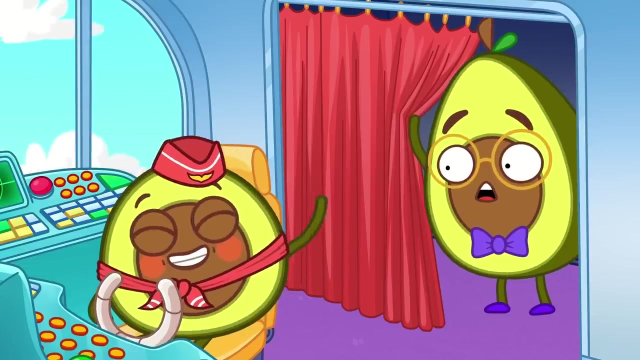 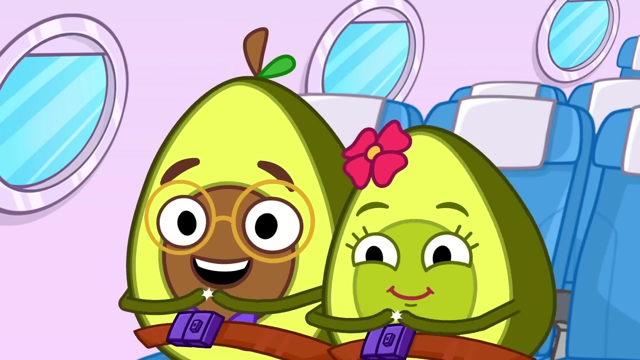 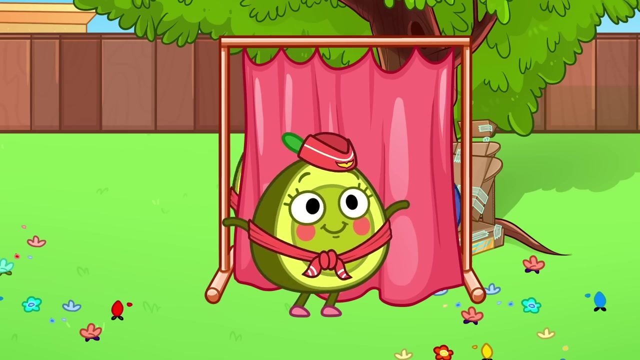 Why is the door locked? If there is a red line on the door, it's occupied. Uh-oh, Who's flying the plane? It's flying the plane. The plane has landed safely. Thank you for flying our airline. You kids were an excellent crew. 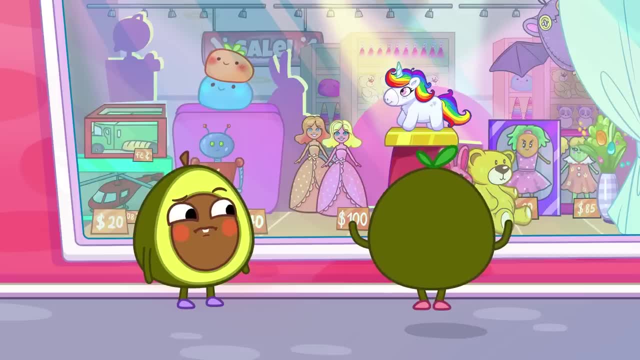 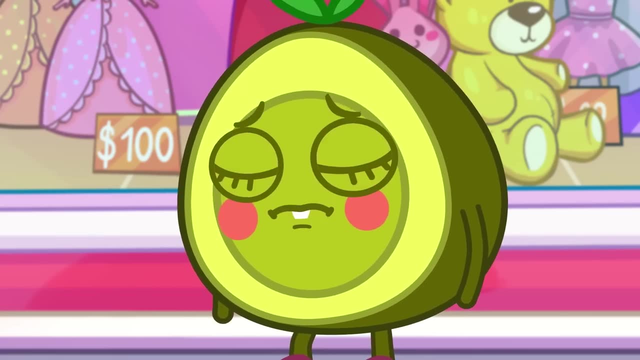 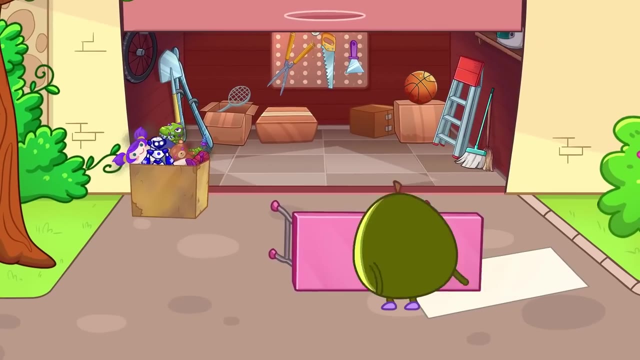 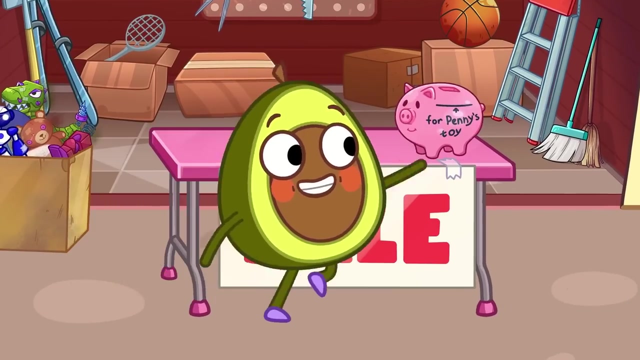 Penny really wants that toy unicorn And Pit wants to buy it for her. But he doesn't have any money. Pit has no money. Pit has an idea. He's going to have a garage sale. He'll use the money for Penny's unicorn. 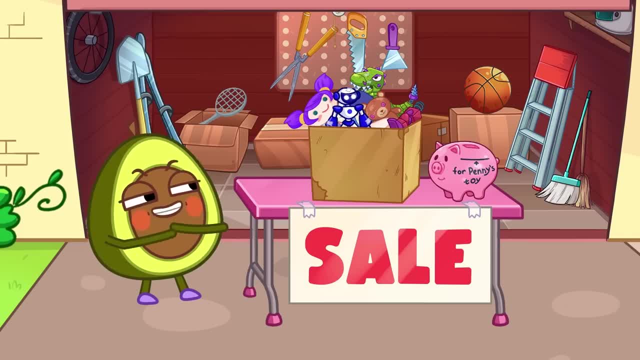 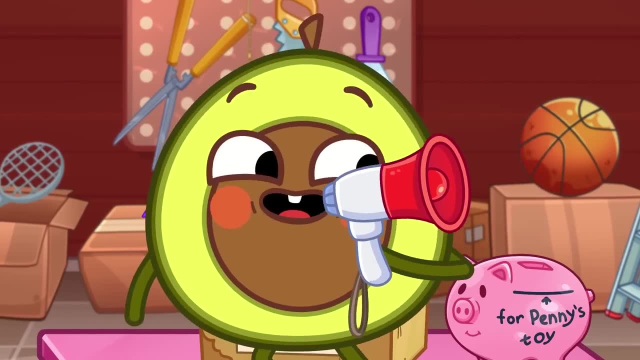 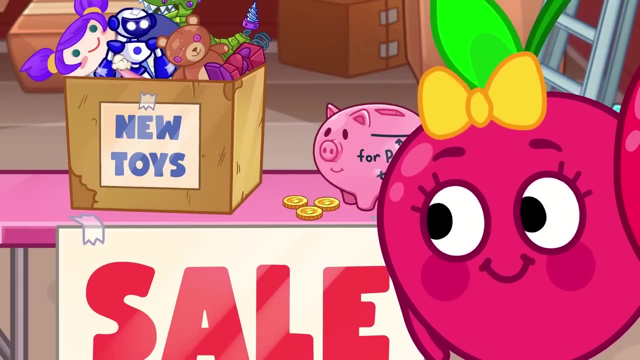 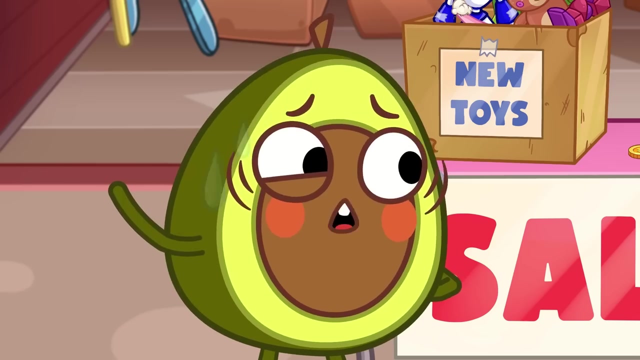 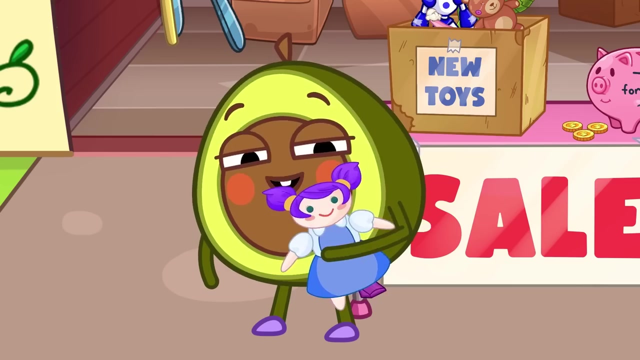 Those toys are old and broken. Pit, New toys. Pit isn't being honest. New toys, New toys for everyone. Maybe Cherry would like a toy. I want a doll. That doll is missing a leg. Just a second Pit. that leg doesn't match. 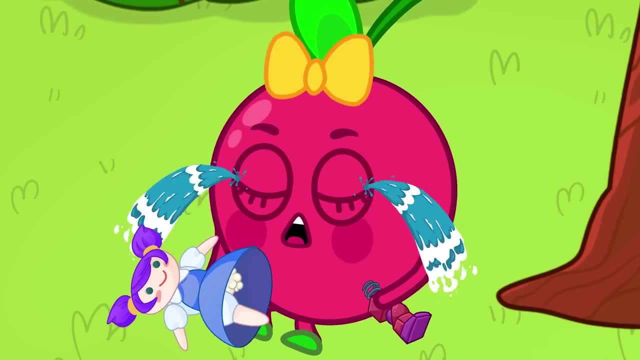 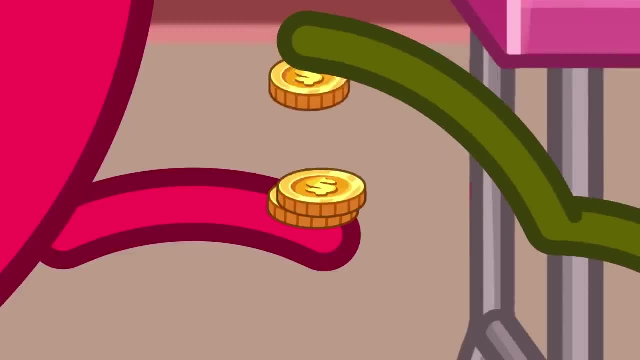 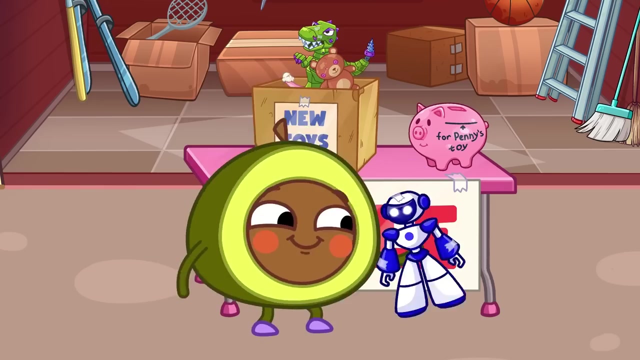 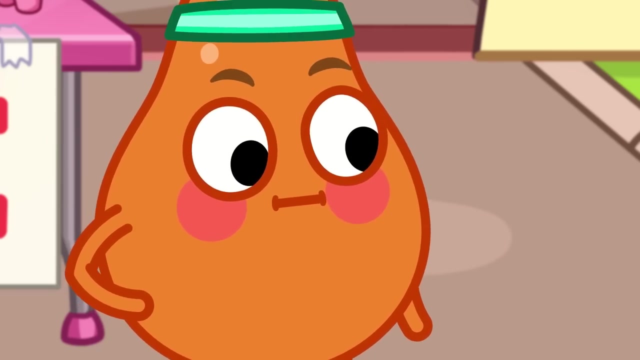 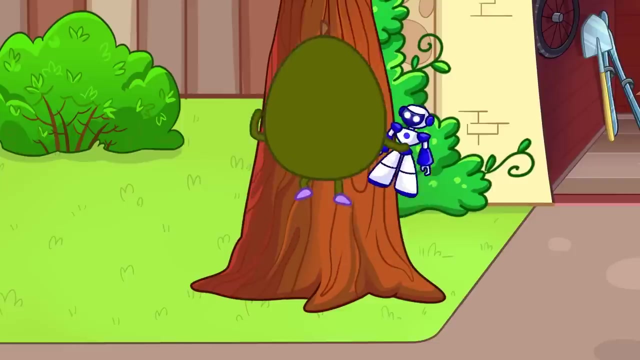 Cherry's crying. The doll's leg came off. Now they want their money back. Maybe Perry will buy something. How about a robot? He doesn't want it. Wait, It can move on its own. That's what I'm talking about. 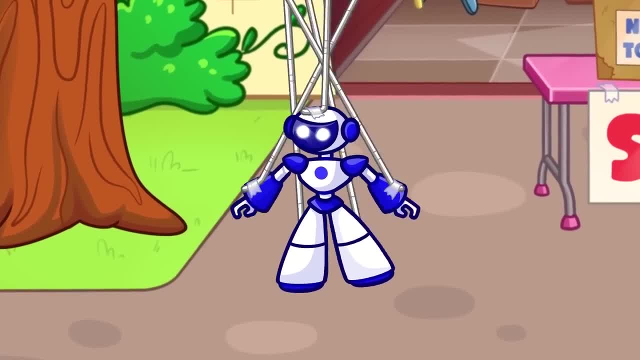 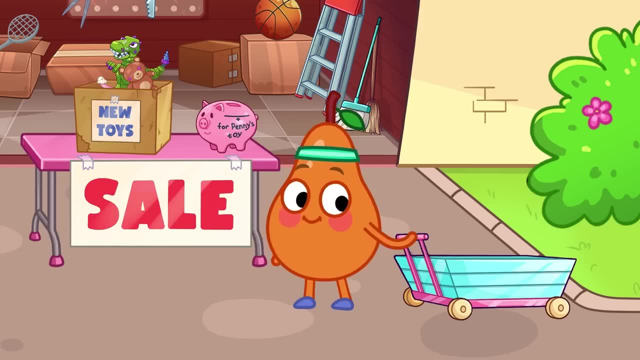 I'm sorry, but maybe it looks like a robot. It's better than a robot. Sorry, I just want it. I know I don't want it. Come on, let's start over. We'll see if I can get it. 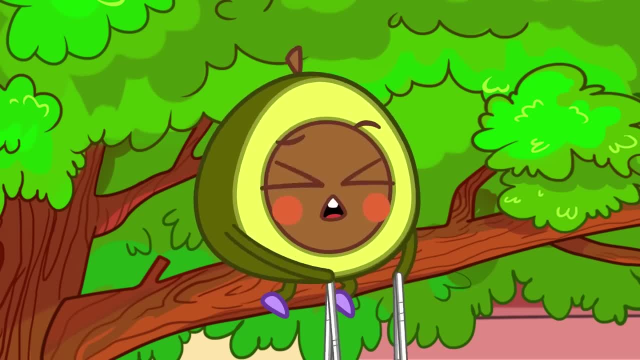 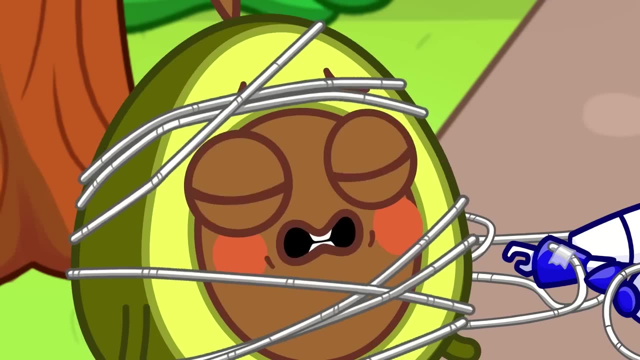 Let's do it Officially. it's a robot And I'm going to start over. Oh, that can't be done. I'm going to start from the start. That's too hard, I can't do it. Come on, let's get it back. 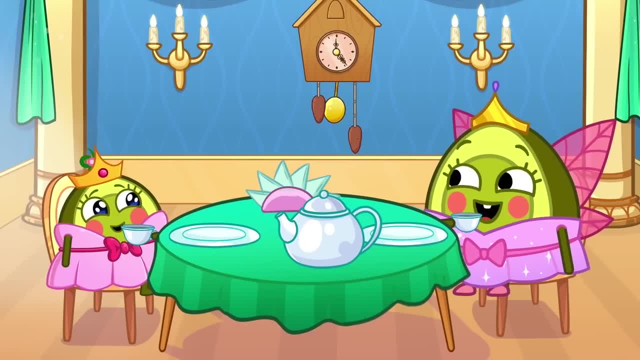 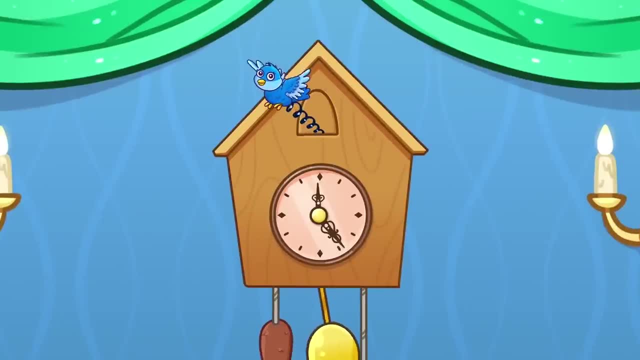 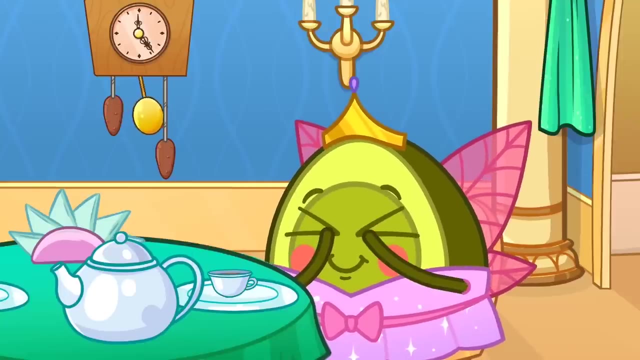 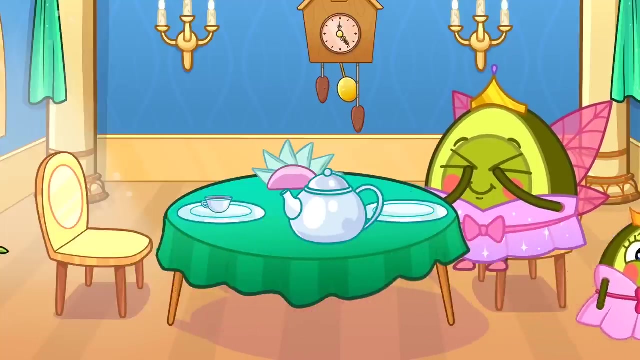 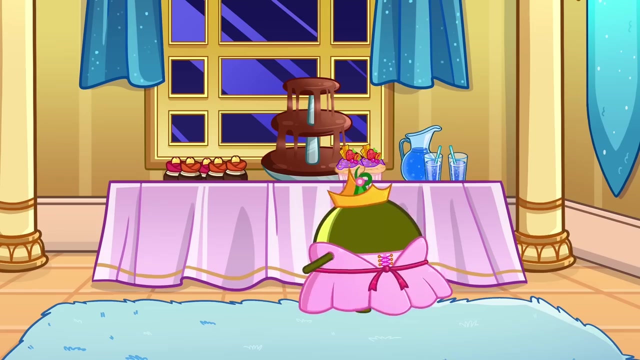 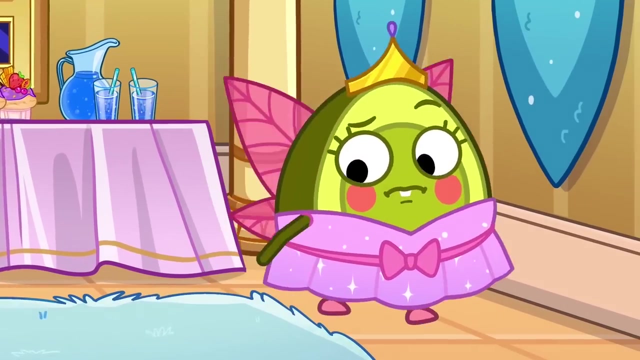 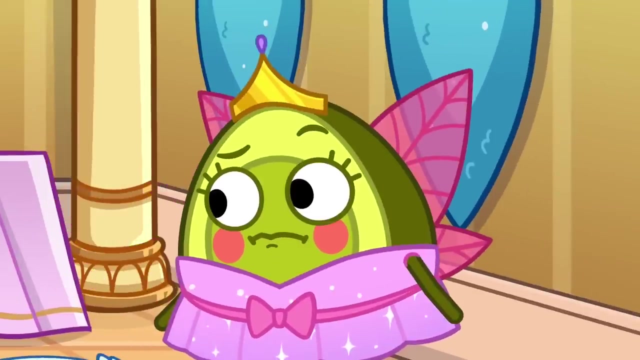 Penny thinks Mommy should have a baby girl. They could have tea parties and play princess. Now what do you want to do, Penny? Penny wants to play hide and seek. Where should Baby hide? Can Penny find Baby? Not there? Not there either. Keep looking. 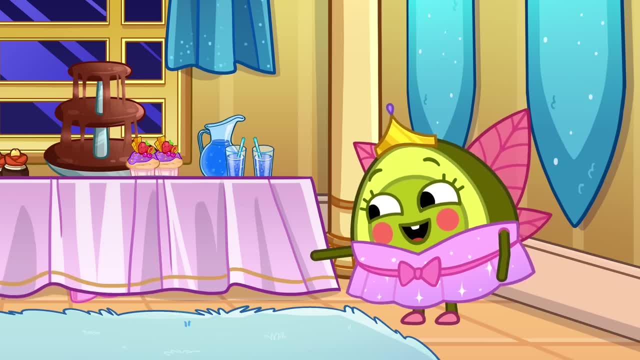 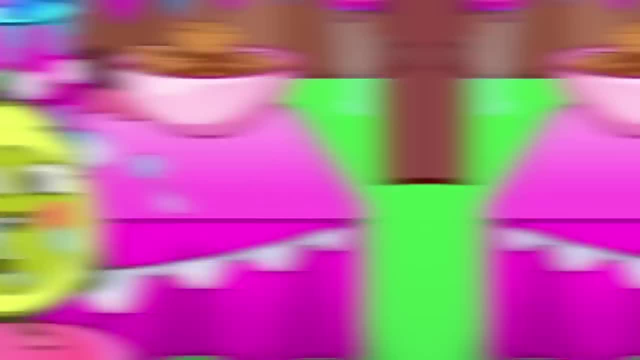 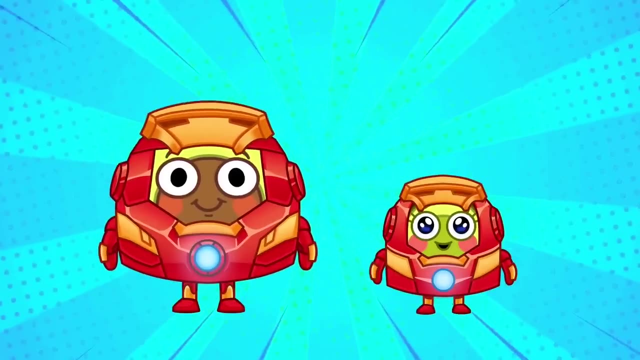 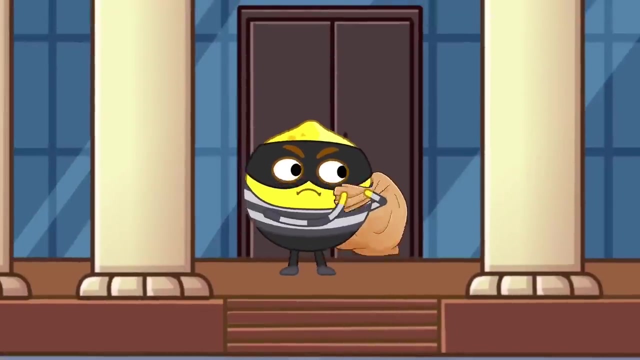 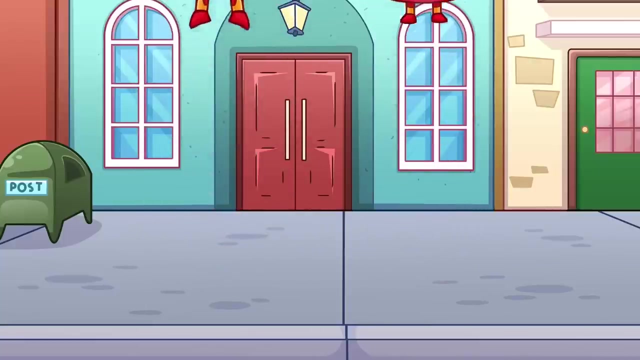 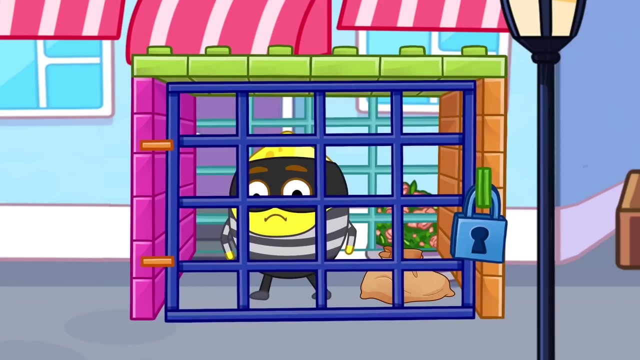 Found you. You're a great sister, Penny. Brrrrr, Huh. Pit thinks Mommy should have a baby boy. Then they can be superheroes together. Oh no, There's a bank robber. Who will stop him? Pit and Baby have saved the day. 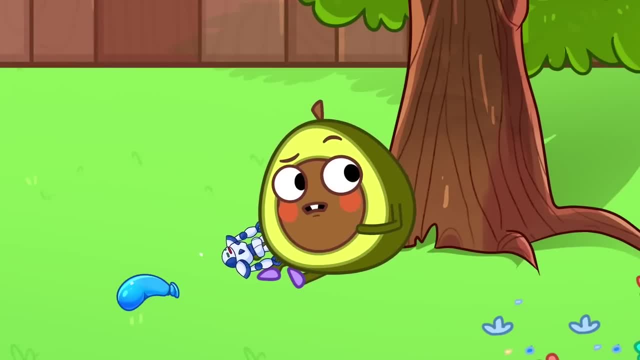 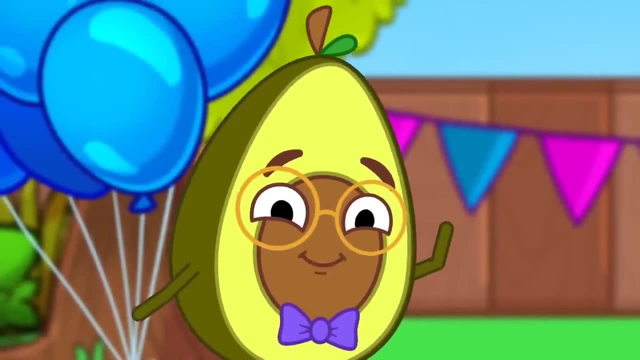 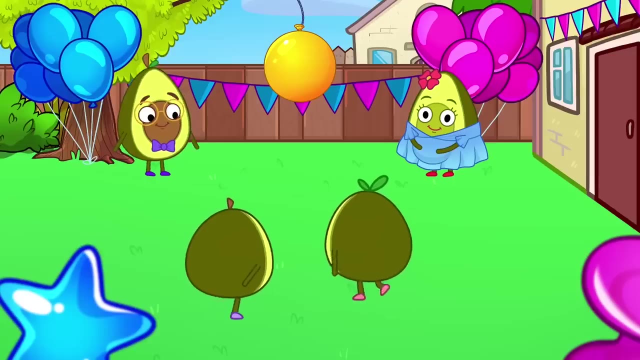 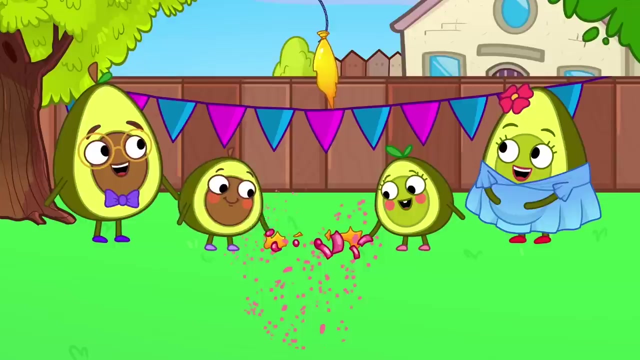 Well done you two. You're a great brother, Pit Kids. let's find out. Are you going to have a baby brother or a baby sister? Find out by popping the balloon. It's pink, which means Mommy is having a girl. 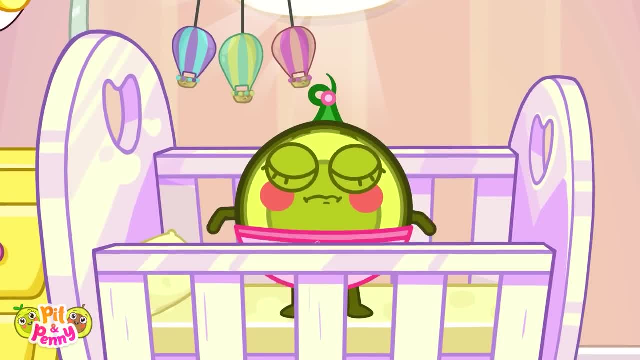 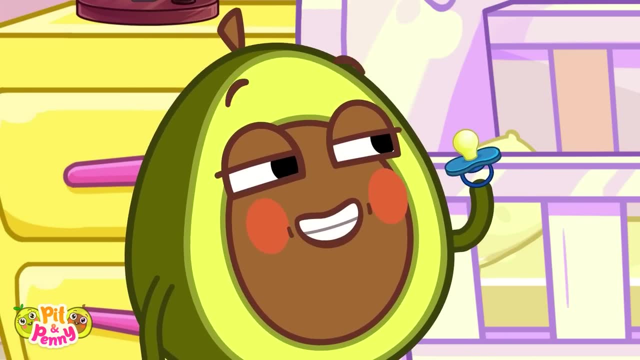 Congratulations. Peppa and Penny are going to have a baby brother. Oh no, Baby is crying. Maybe she wants her pacifier, Or maybe she wants a pacifier That didn't work. No, No, No, No, No. 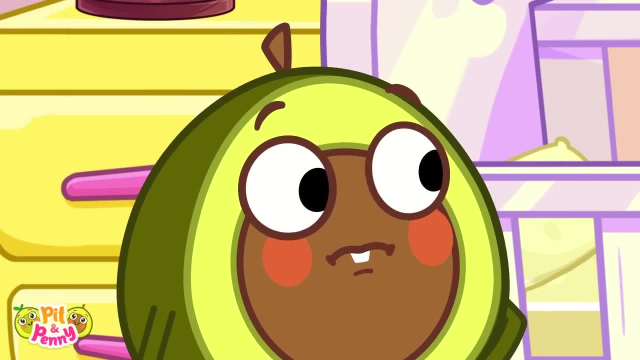 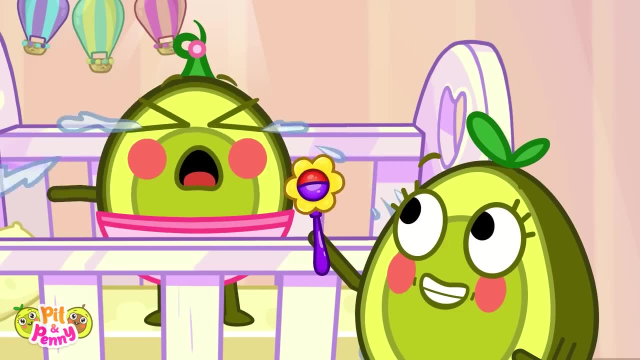 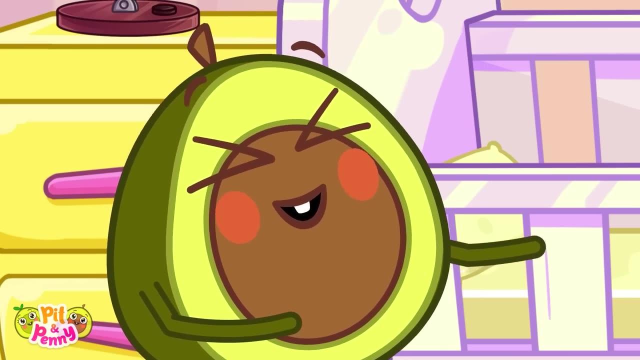 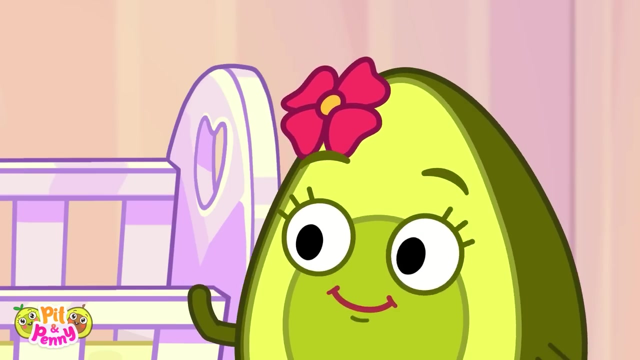 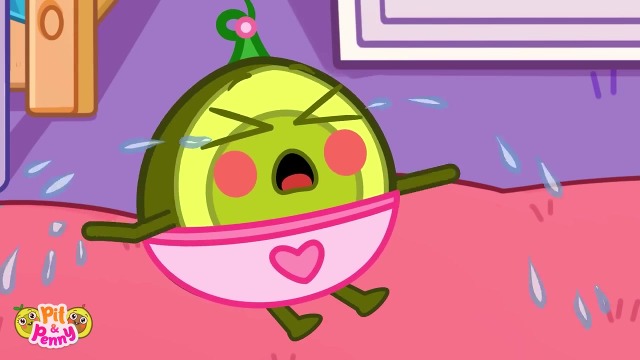 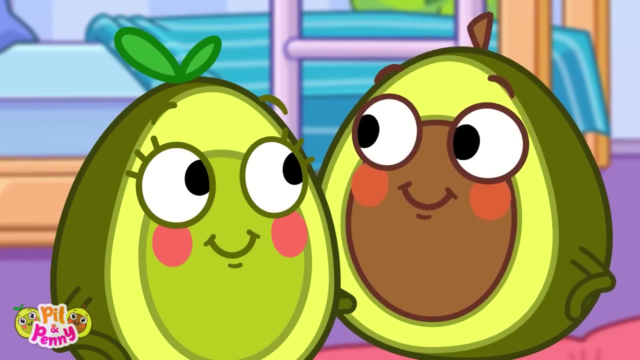 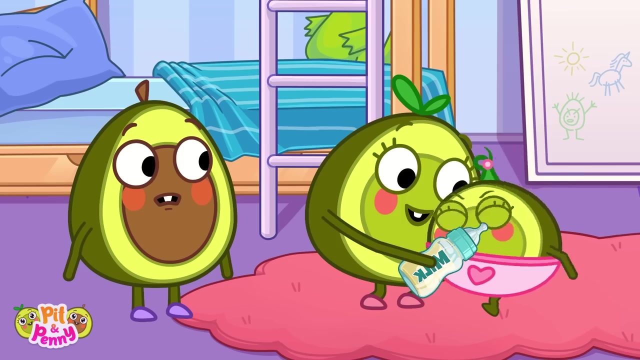 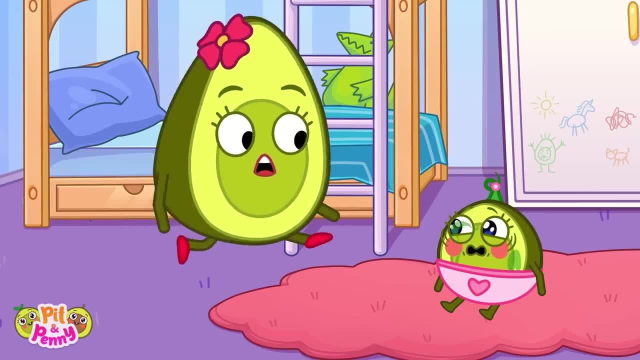 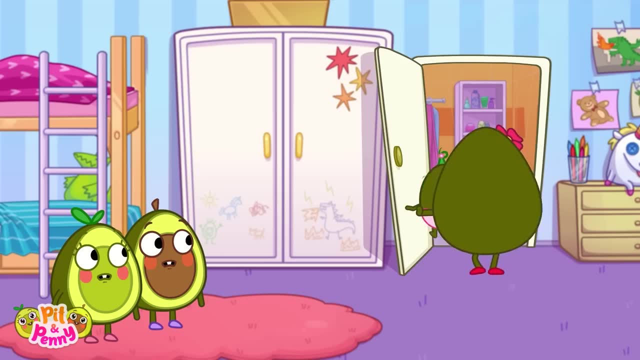 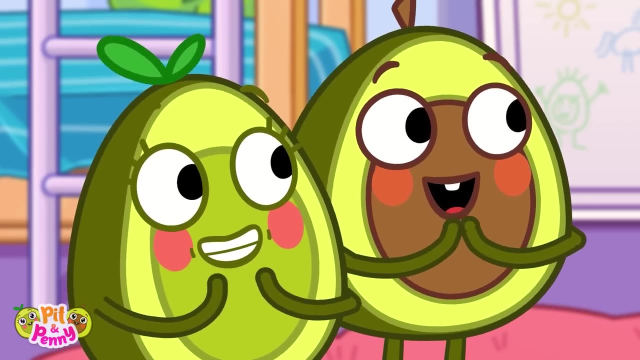 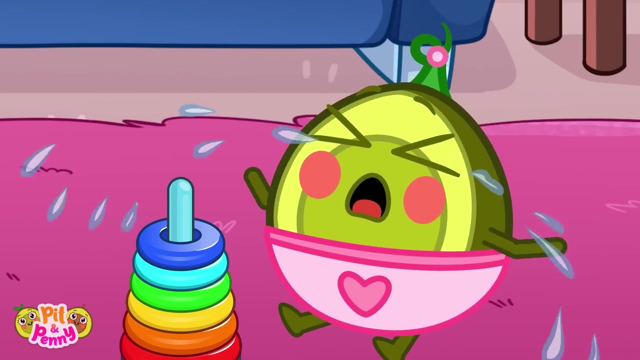 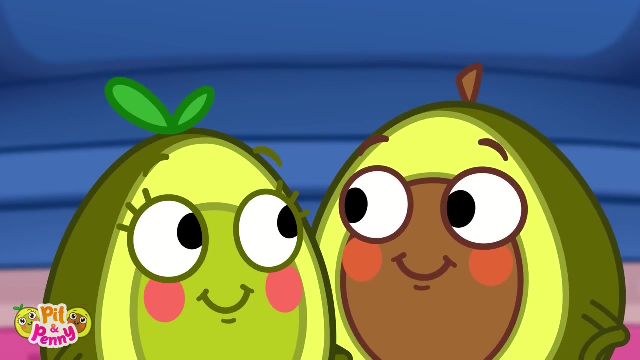 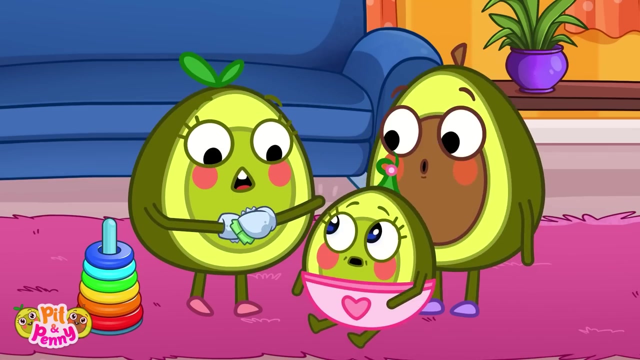 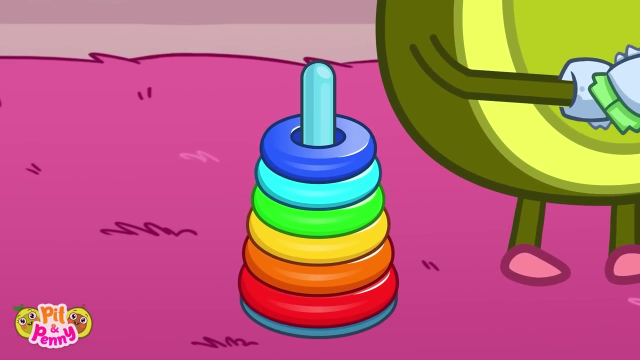 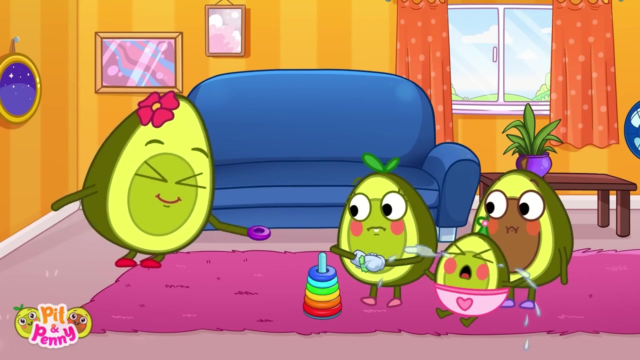 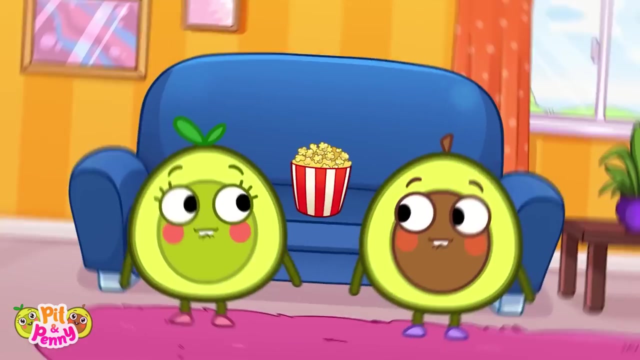 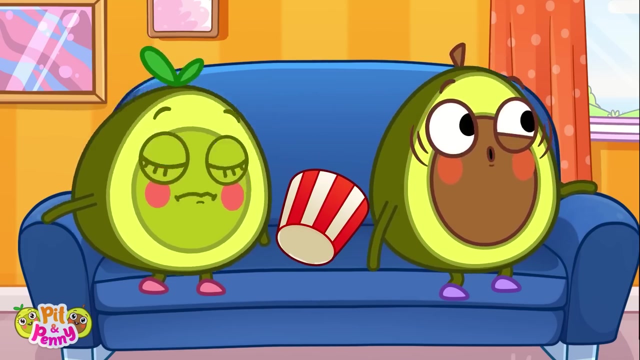 I think she has a dirty diaper. Baby feels much happier. Baby's crying again. Now why is Baby crying? Pit thinks she needs another diaper change. Can you help, Mommy? It's the ring Baby lost. Baby is happy again. Yep, Baby is crying again. 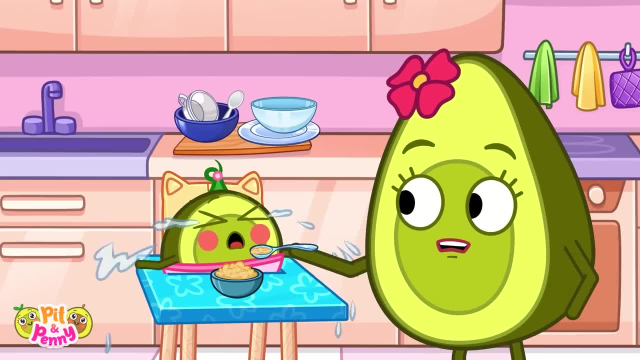 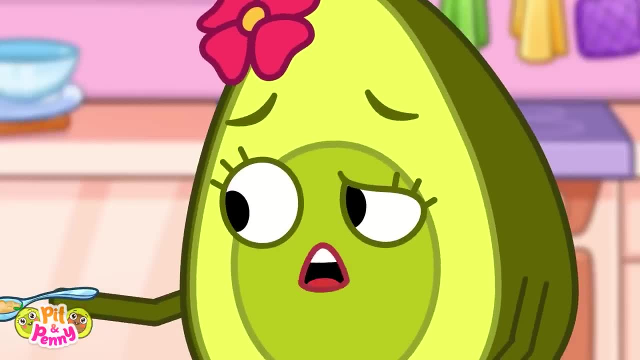 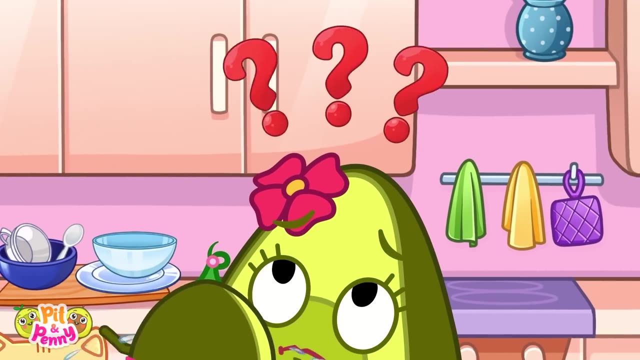 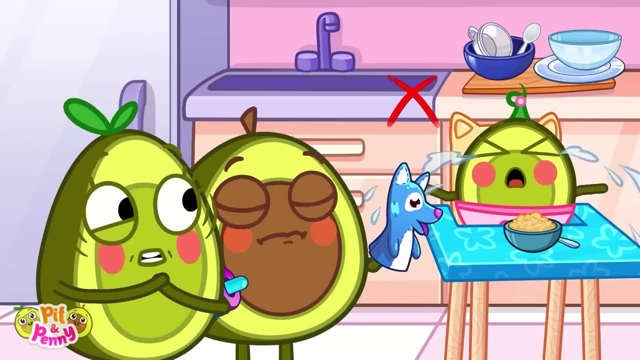 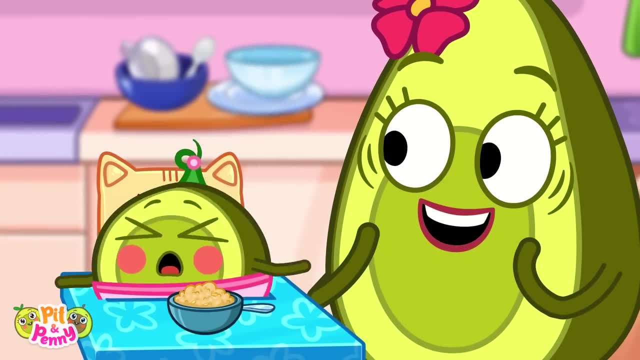 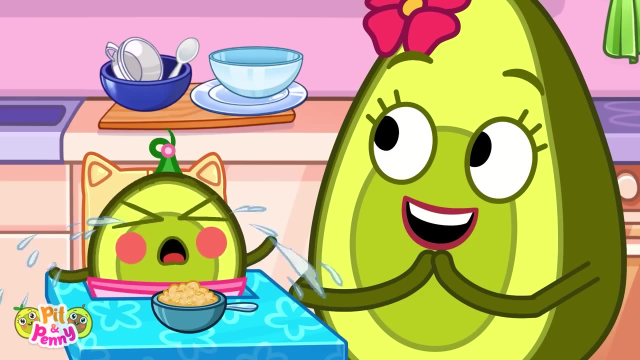 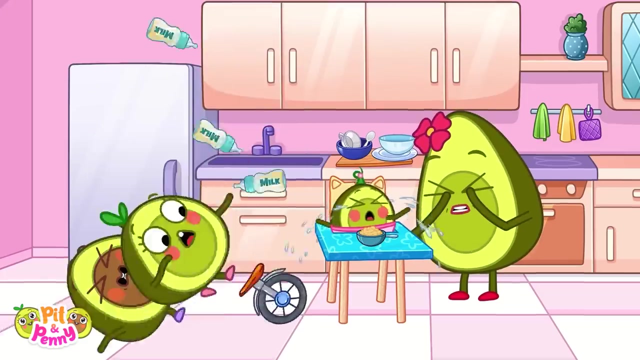 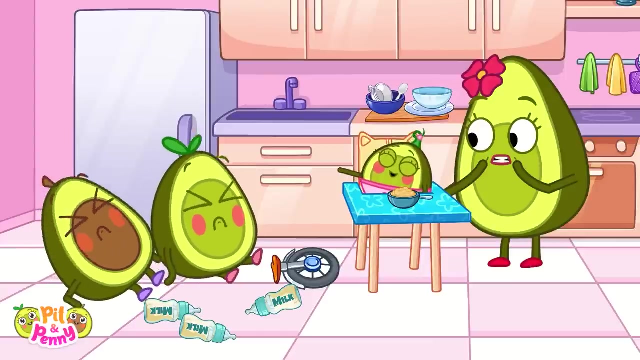 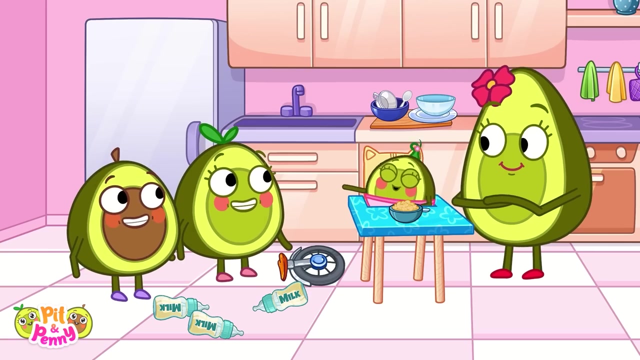 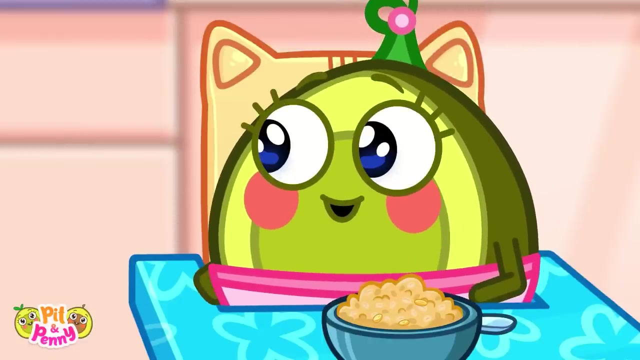 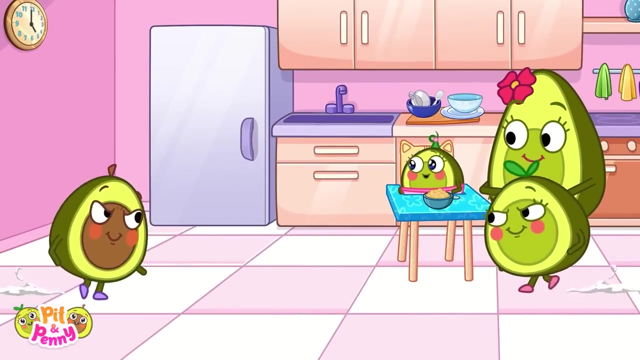 Maybe she wants a puppet show. Maybe she wants to see Pit and Penny juggle. But be careful. Pit and Penny Falling down made Baby laugh. Hit pretends to fall, Penny pretends to fall And Mommy pretends to fall. 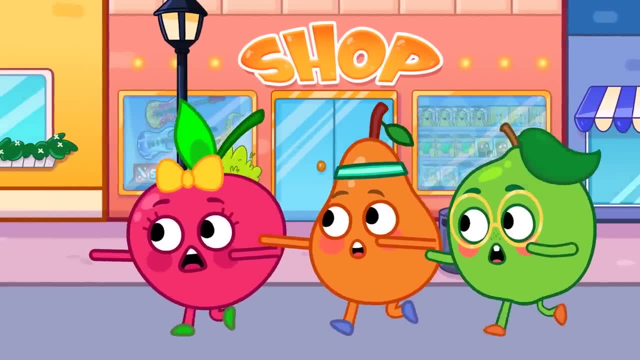 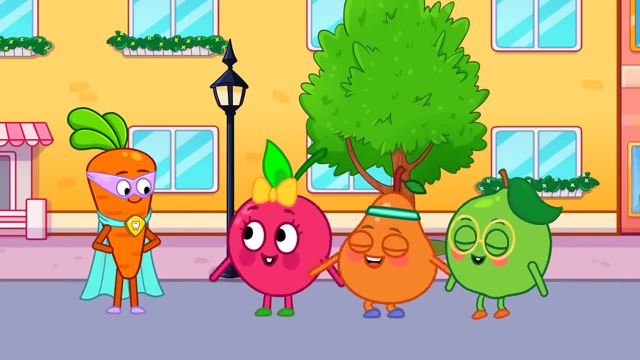 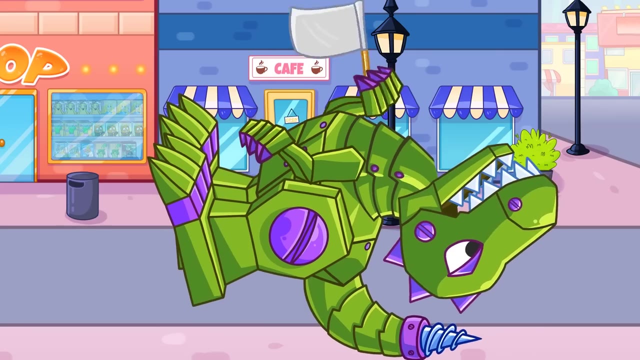 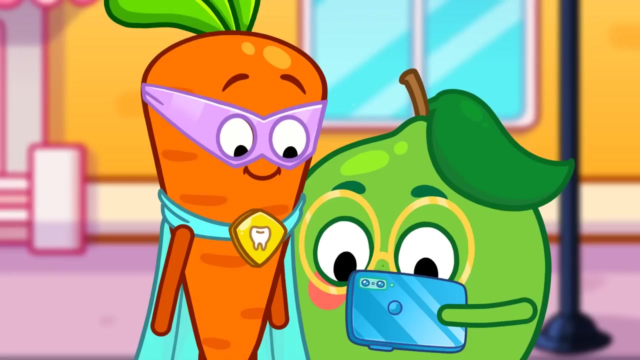 Have fun everyone. Have fun everyone. Oh no, Who will save the children? It's Super Carrot, And he's just in time. Super Carrot saves the day. Thank you, Super Hero. Carrot Say cheese, Oh. 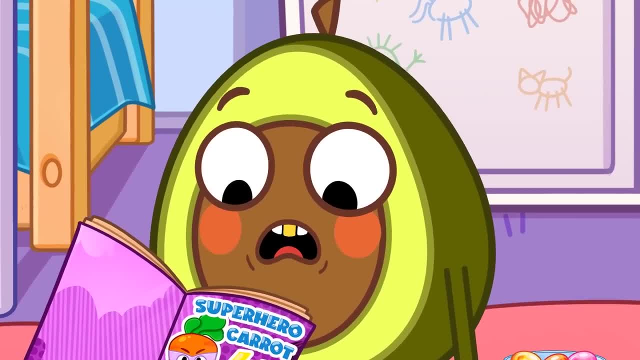 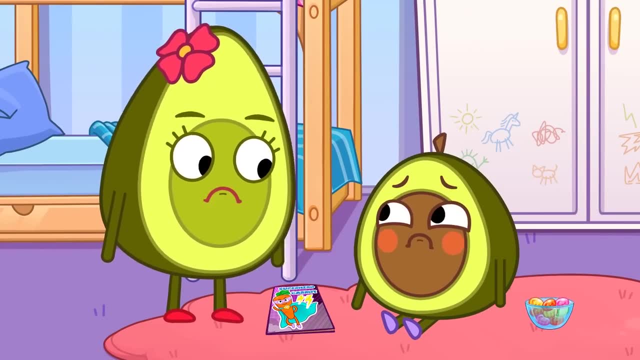 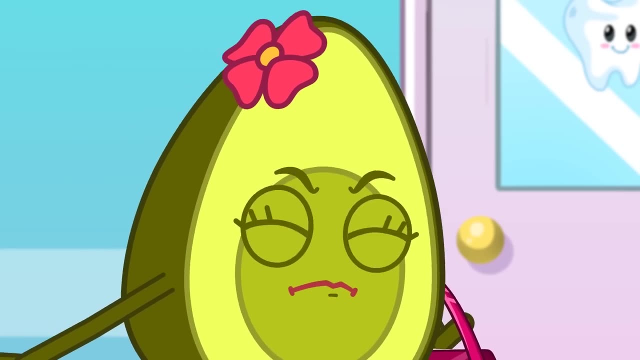 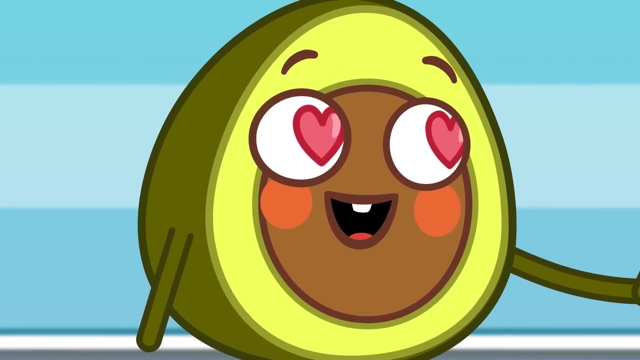 It was just a story in Pit's favorite comic book. Pit has a cavity. What do you think, Mommy? We need to go to the dentist. Pit is afraid of the dentist. Maybe reading your comic will help, Okay, Yay. 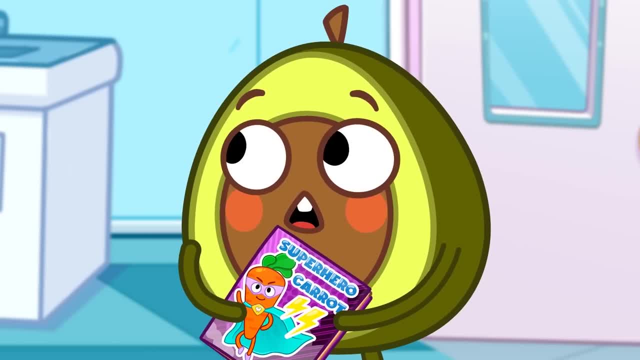 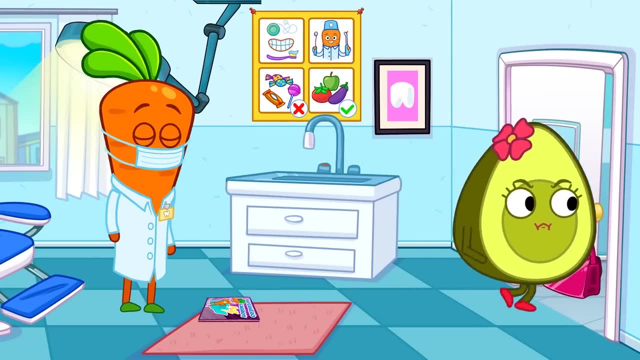 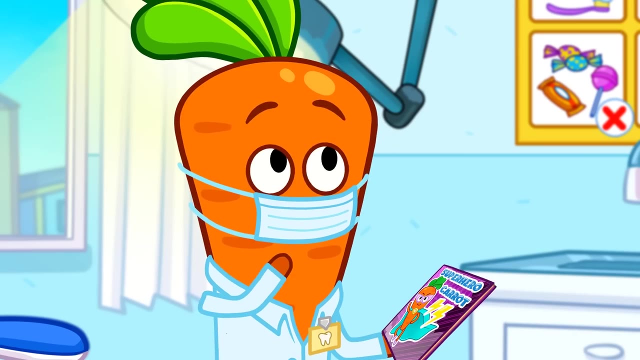 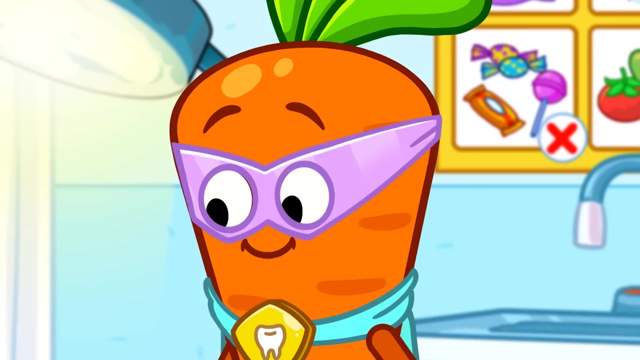 Hello Dr Carrot. Please come in. This isn't good news. Pit thinks Dr Carrot is scary. Sorry, Dr Carrot has an idea. Look who's here. Pit Pit is no longer scared of the dentist. 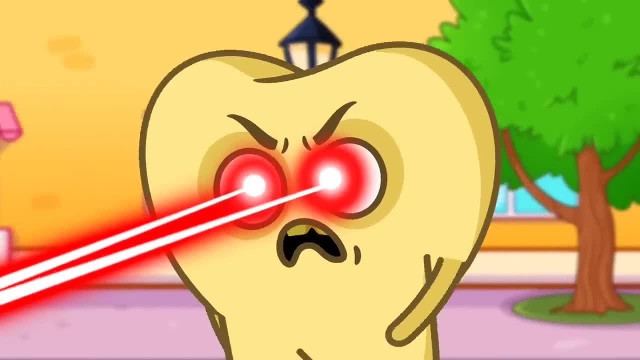 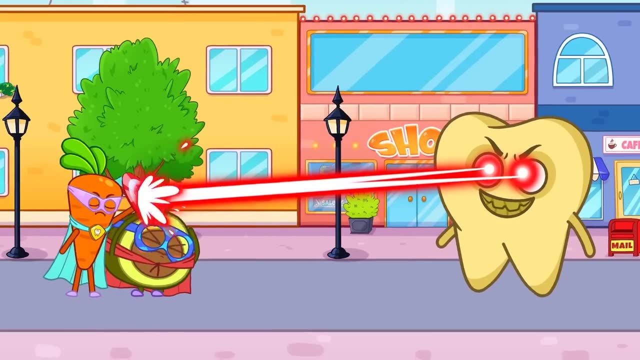 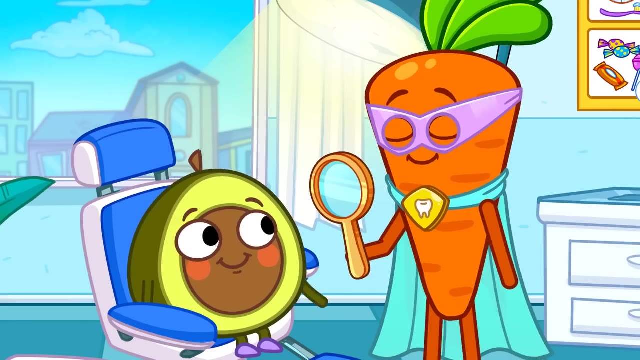 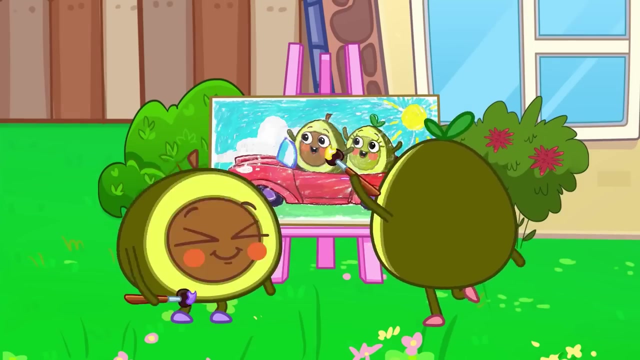 Who will save the children? this time It's Super Carrot and Pit. The evil tooth didn't stand a chance. Smile, Pit, Your cavity is gone. Dentists can be super too. What a wonderful picture. Someone erased the color. 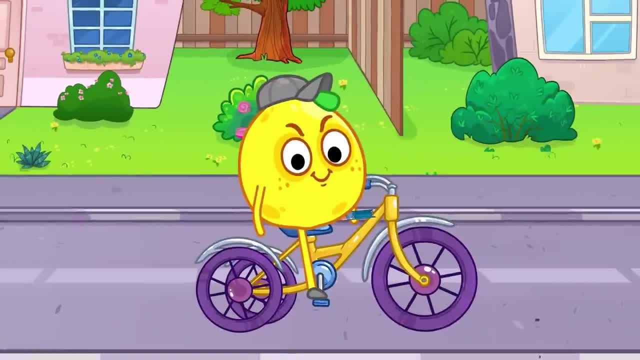 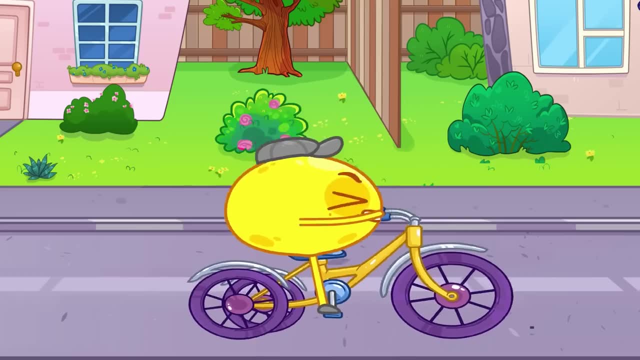 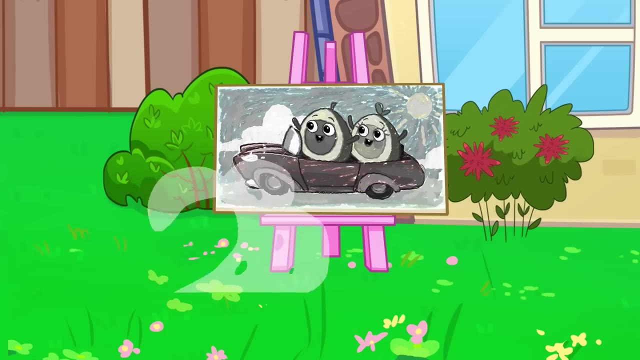 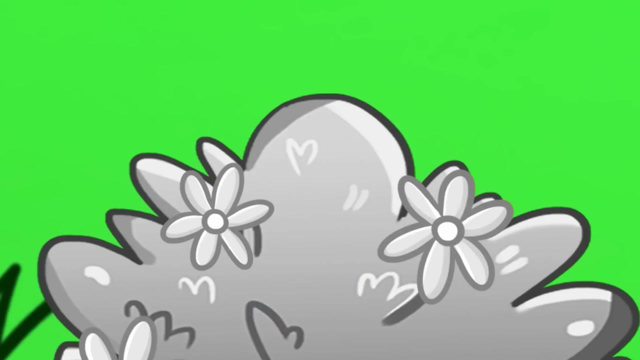 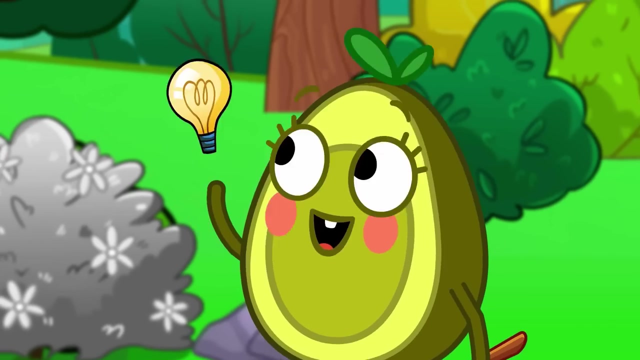 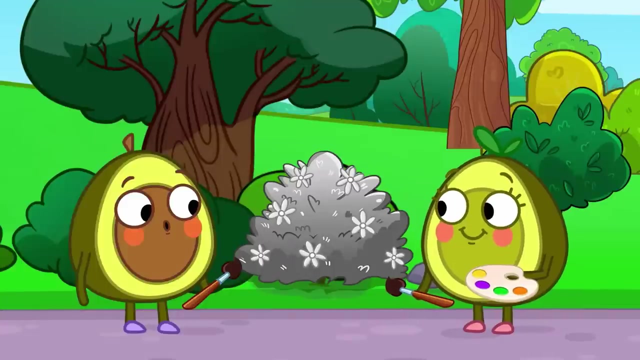 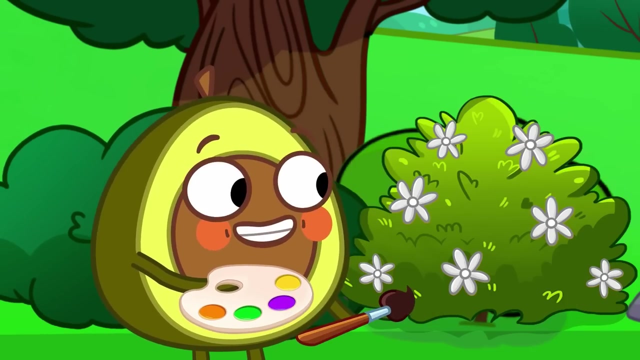 It was Little Lemon. He has a magic eraser. Wait, He stole the color from the bush. Can you hear me Fix it? Pit and Penny, They'll paint the color back: Green for the leaves And the yellow for the flowers. 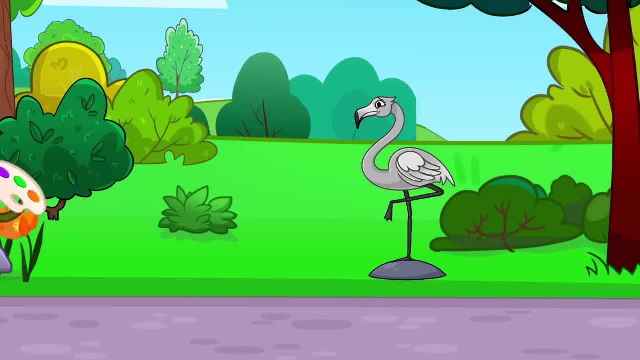 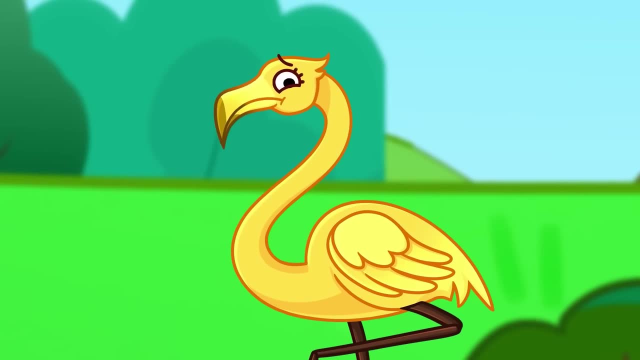 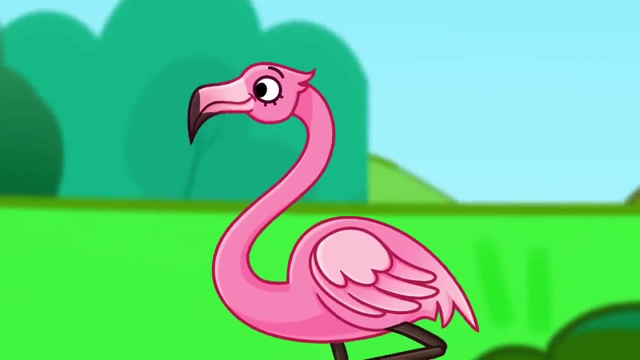 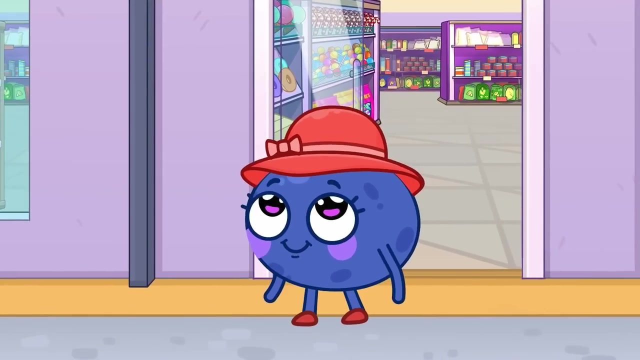 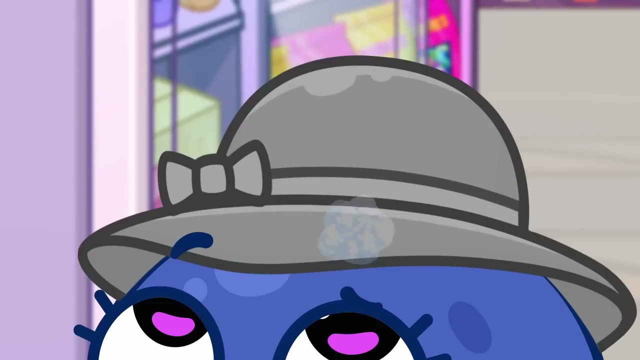 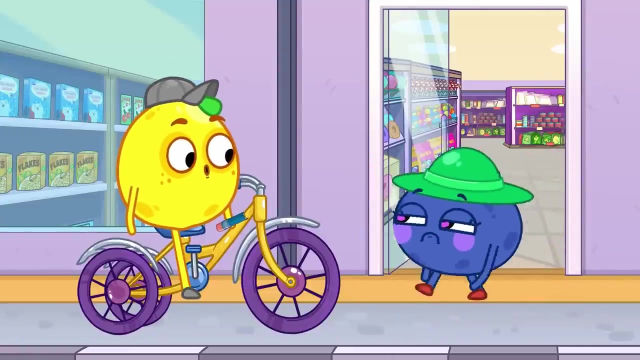 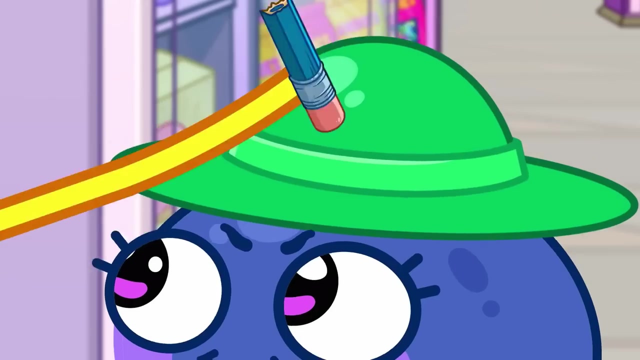 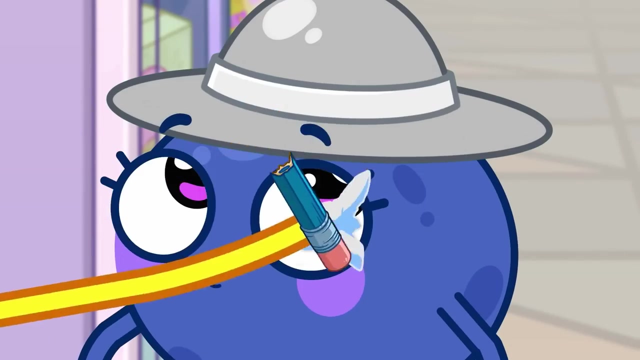 Oh, no, Poor Flamingo. The flamingo needs some color. Yellow is the wrong color. Yes, Flamingos are pink. Watch out Blueberry. Ha ha, ha, Huh, She gets it. Blueberry's color is. 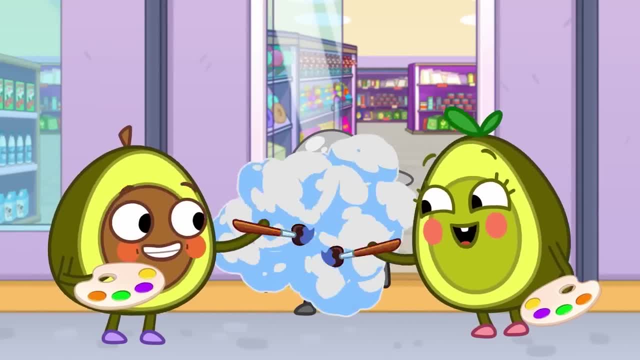 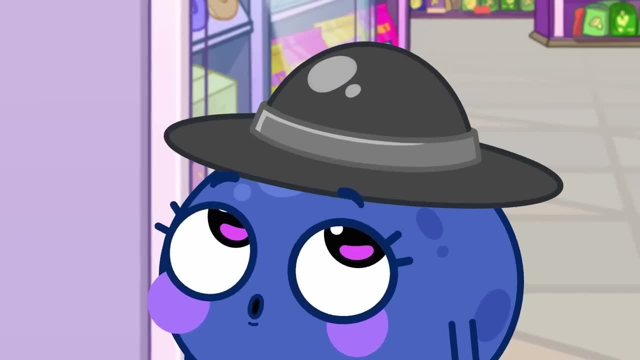 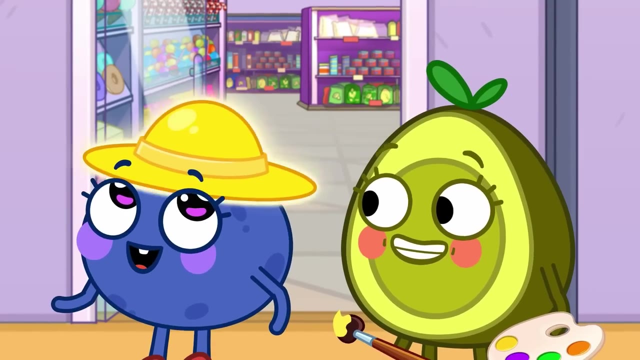 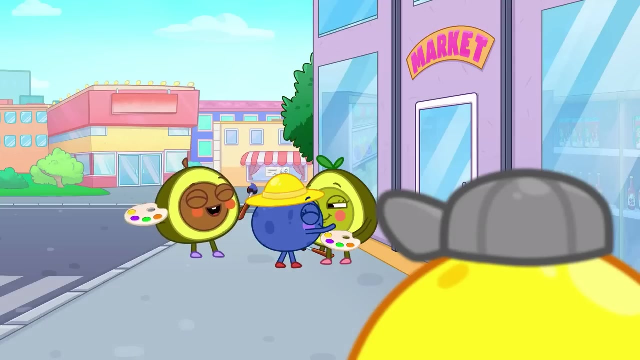 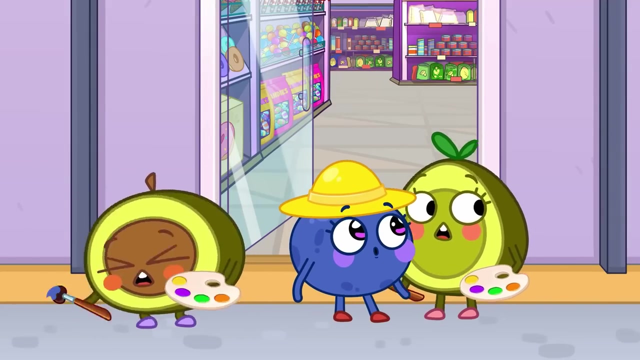 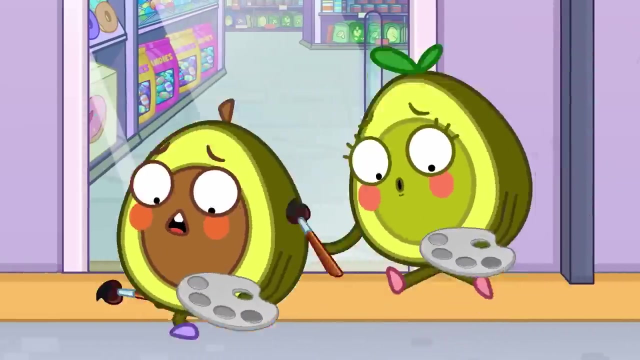 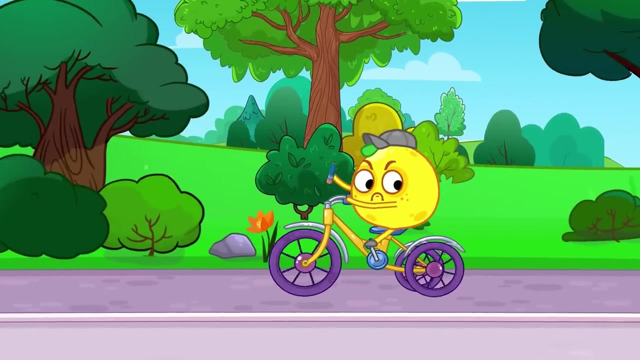 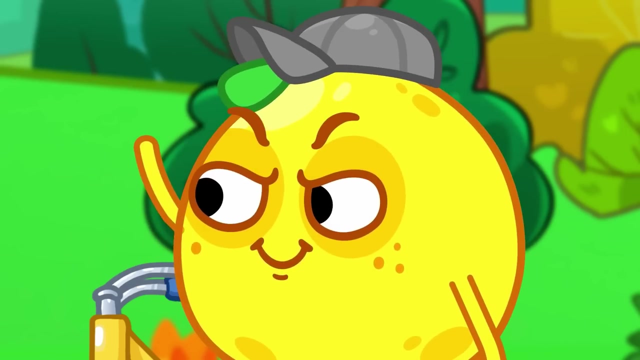 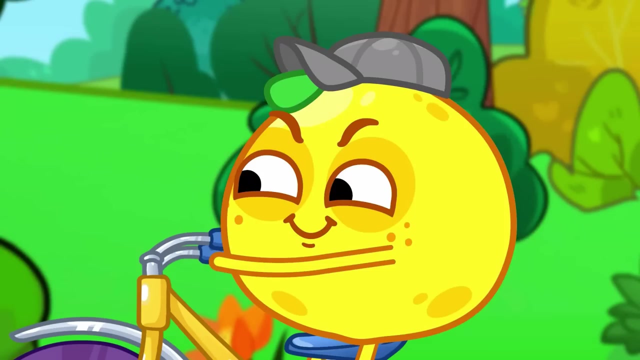 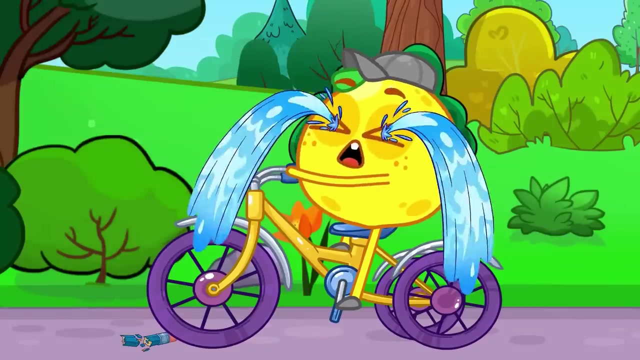 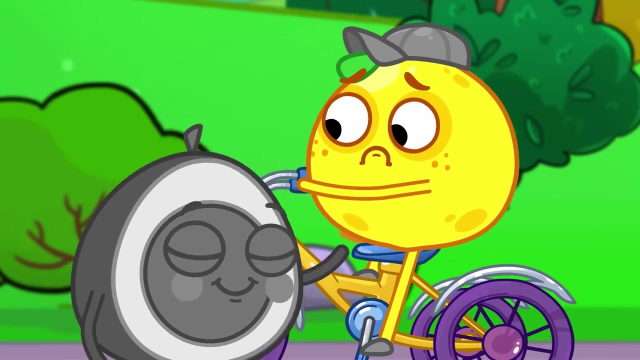 Green. Pit and Penny will fix it. That's too dark, That's much better. Yay, Little Lemon isn't very happy. Run kids. Pit and Penny are great And the magic pencil is broken. Pit knows what to do. 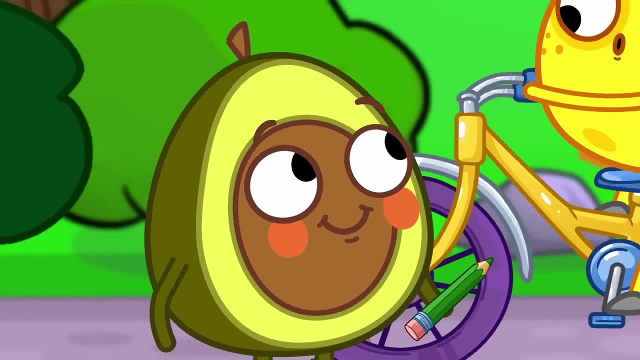 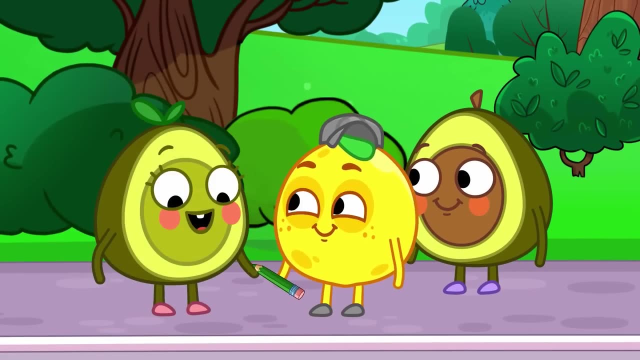 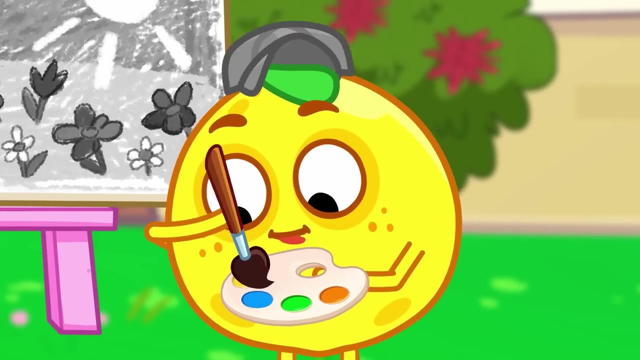 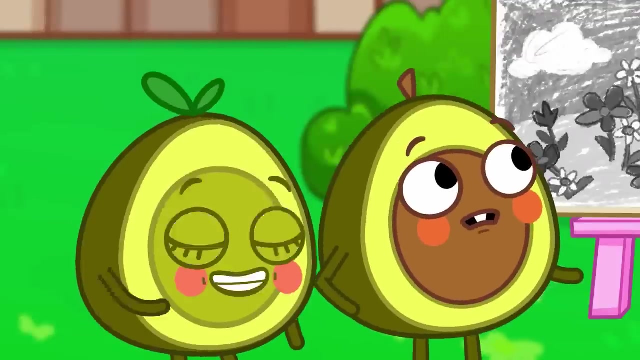 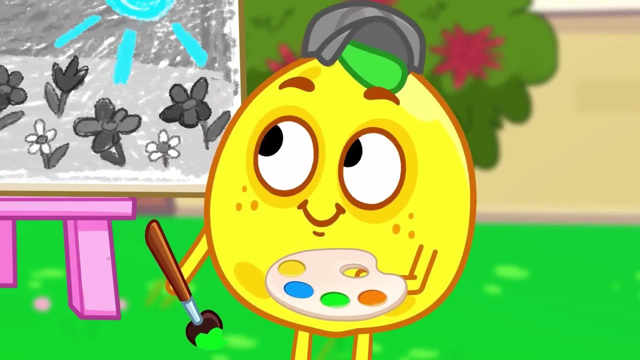 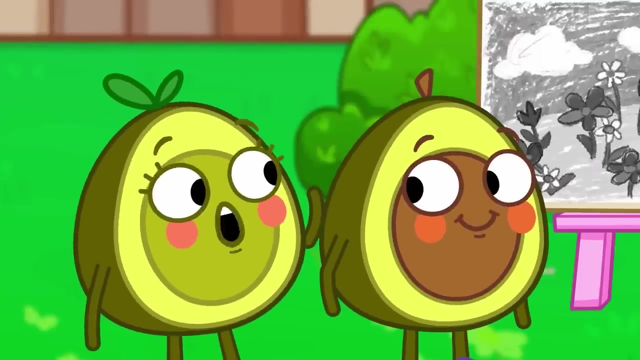 Painting things is much more fun. You try Little Lemon. Well done. The sun isn't blue. Try another color. It's not green either. Help him, Penny. The color of the sun must be warm, Just like you. 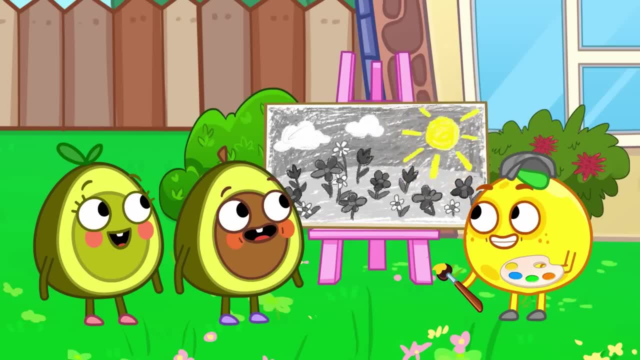 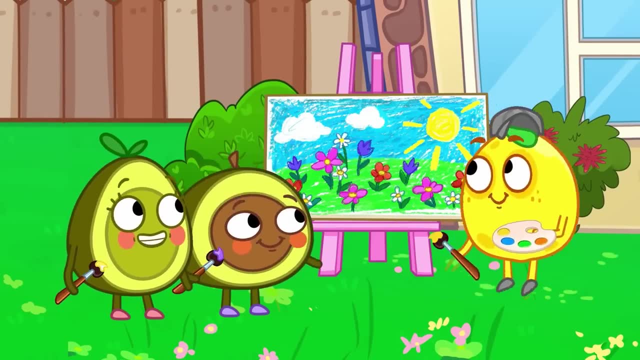 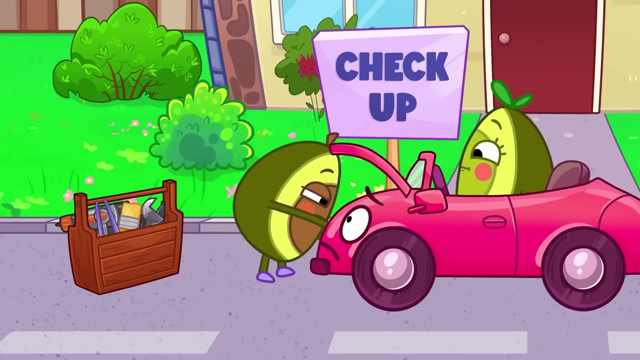 The sun is yellow. Good job, Working together is a lot of fun. Blue car is nervous. It's his turn next for a checkup. Paint car is as good as new. Your turn. Blue car. Pit just needs the pliers. 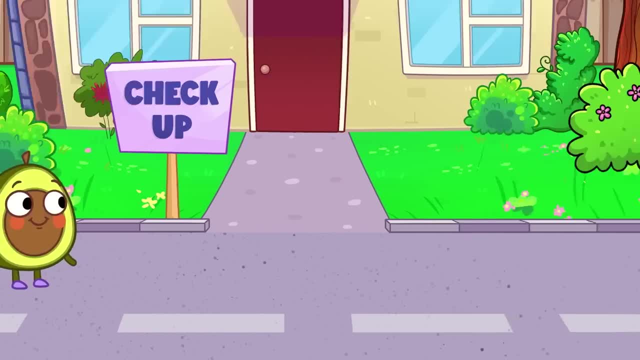 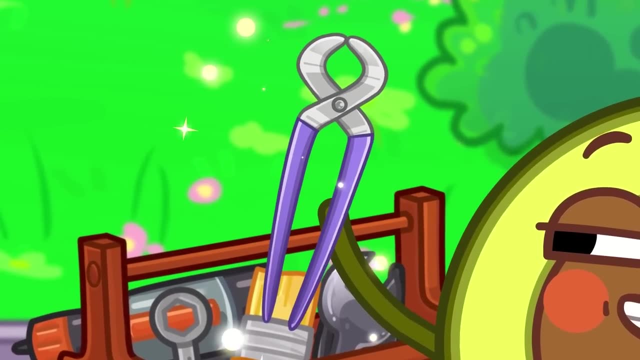 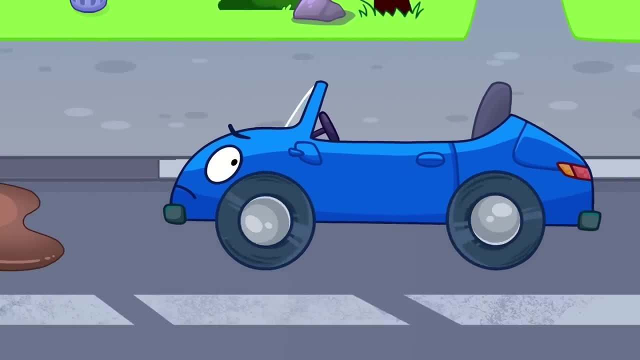 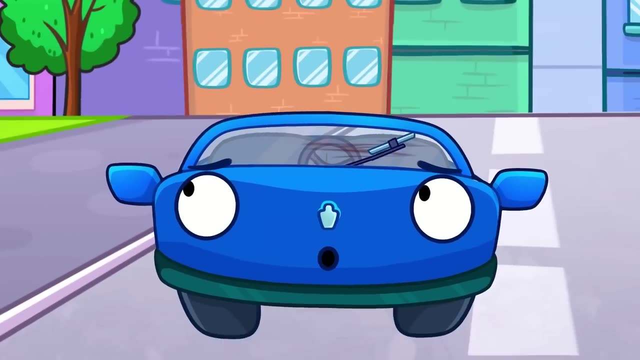 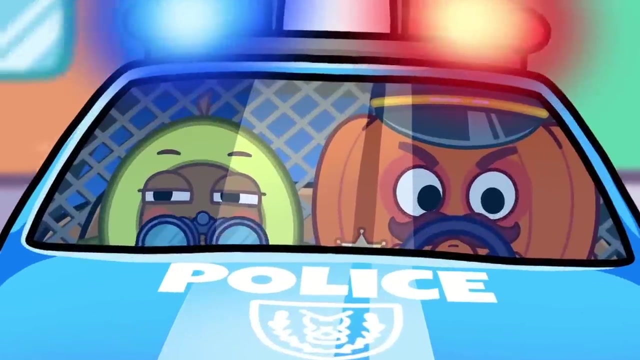 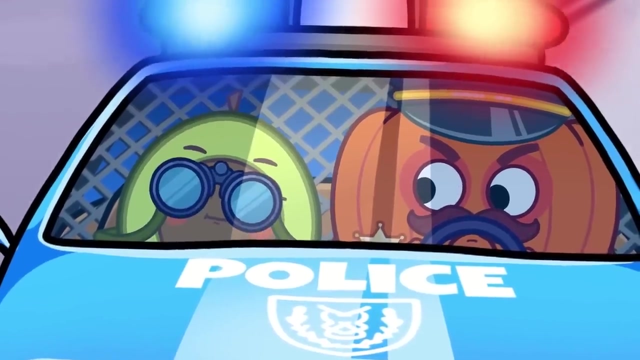 I'm going to get you. I'm going to get you. Blue car is running away. Oh no, He lost a windshield wiper. Here come Officer Pumpkin and Pit. Blue car is hiding in the tunnel. There's the windshield wiper. 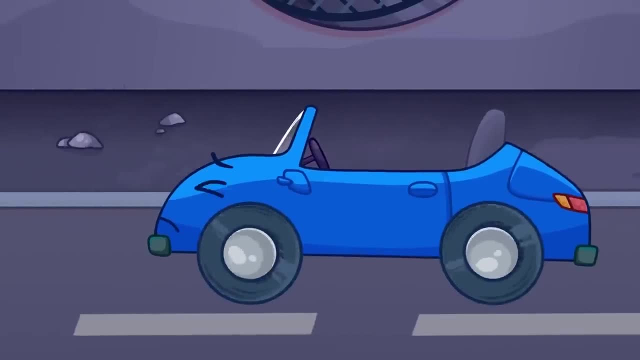 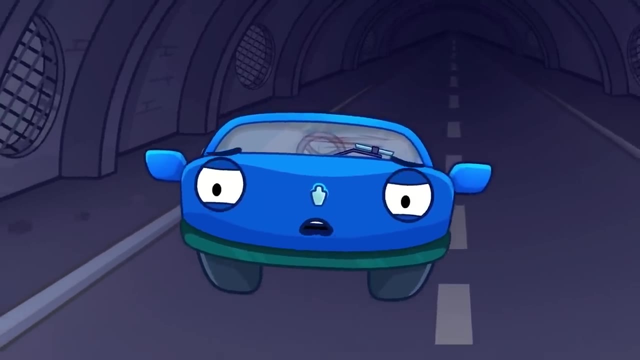 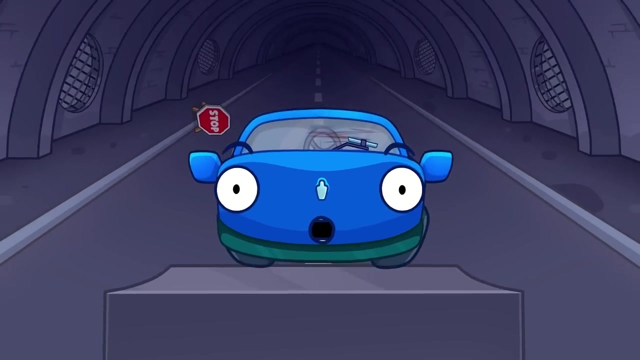 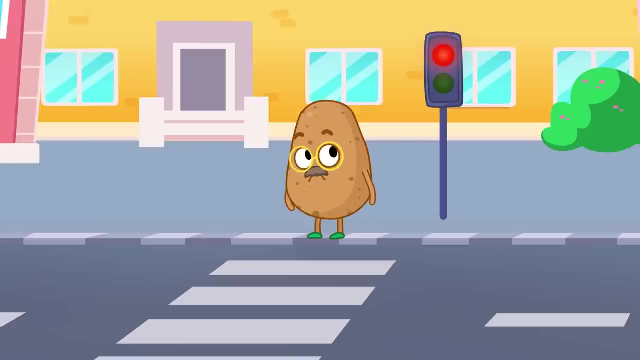 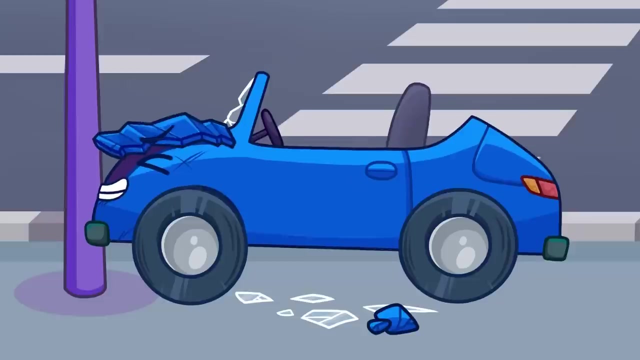 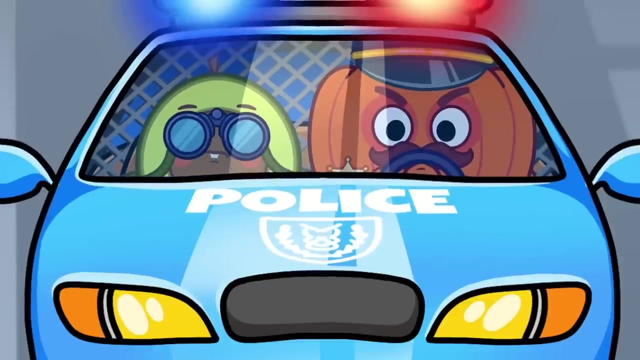 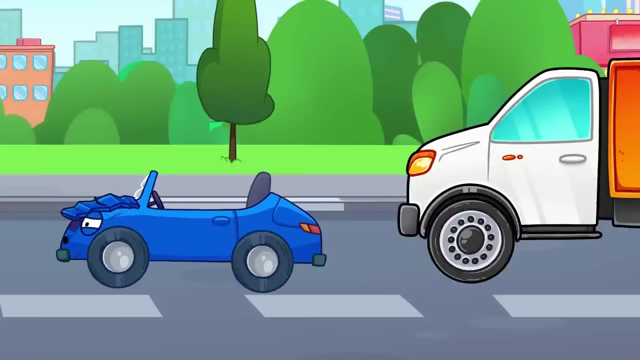 My car was here. The tunnel is dark and scary. I can't see anything. He didn't see the stop sign. Poor blue car. Blue car hit the lamppost. Another clue for Pit to follow. Blue car lost a tire. 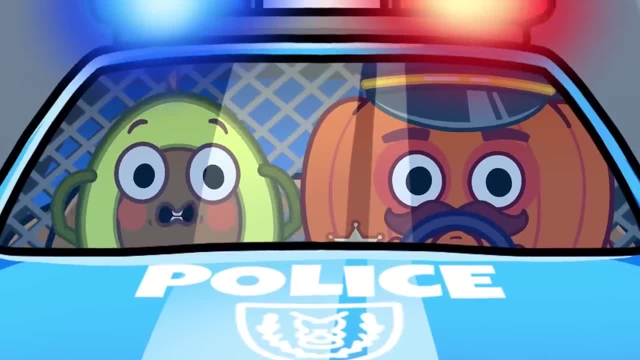 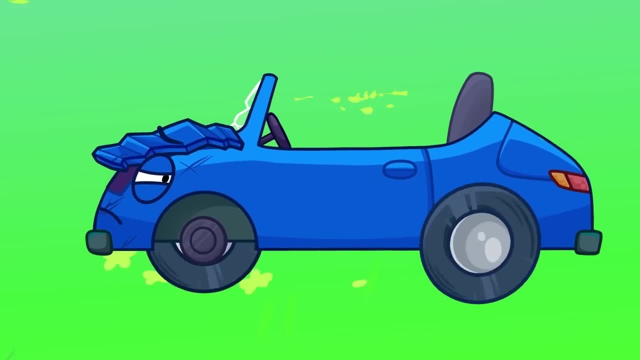 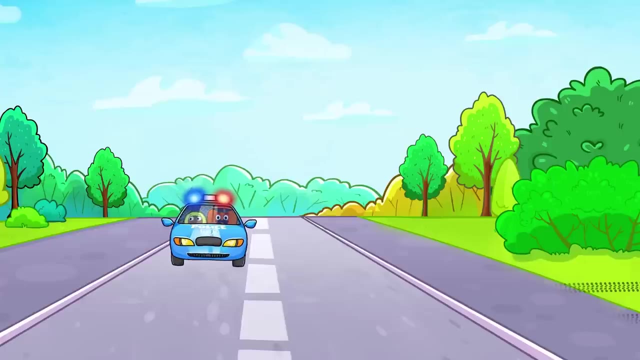 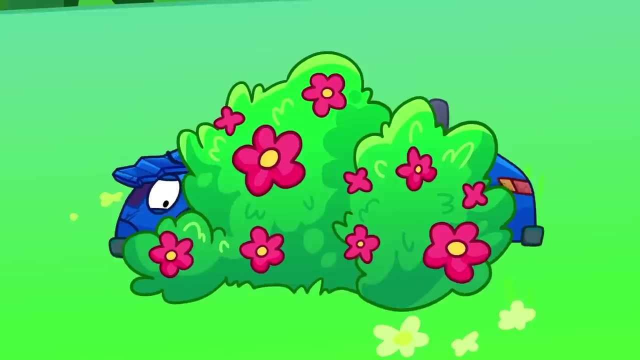 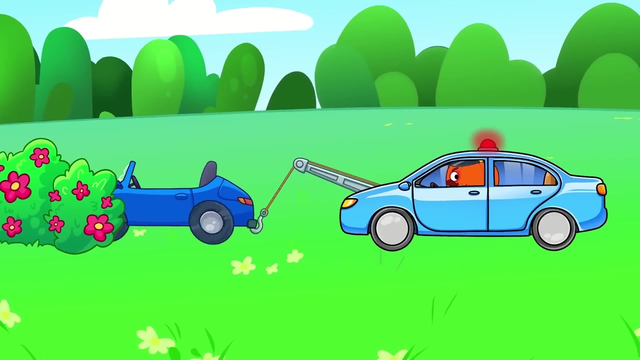 Oh no, This is a tweez. Watch out for the tire. And now blue car is stuck in a bush. Hurry, He's over here. There it is, Let's go, Let's go, Let's tow the car to safety. 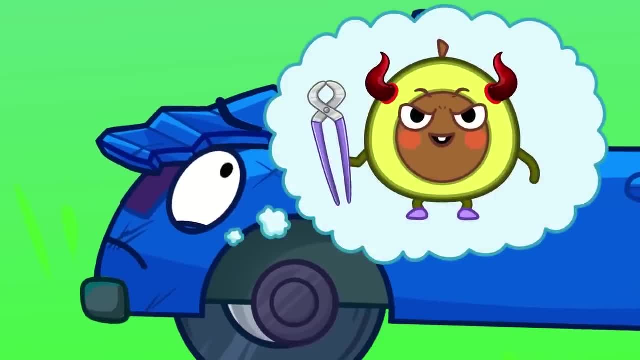 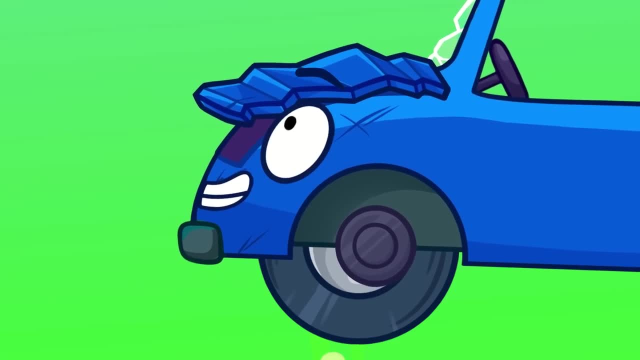 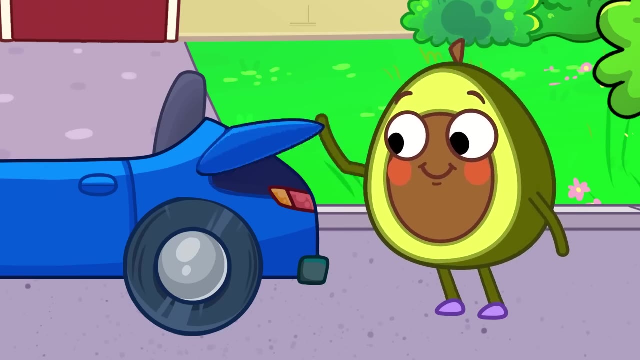 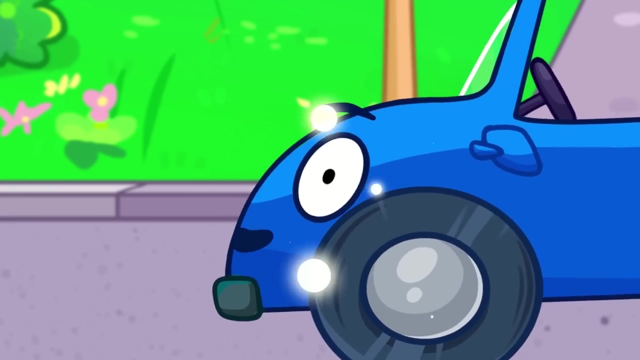 I'm afraid of checkups. Checkups are necessary so that you don't get into an accident, Just like going to a doctor Time for a new battery- See blue car. Checkups are easy Now. I will never be afraid of checkups. 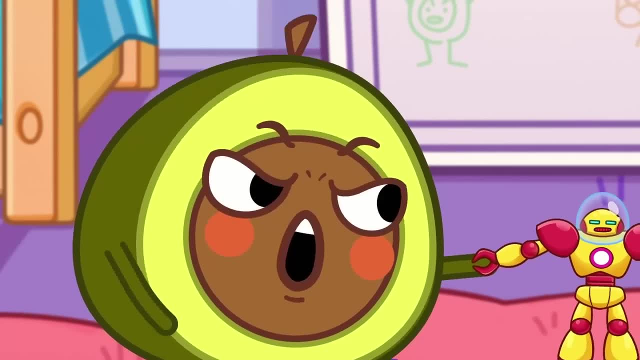 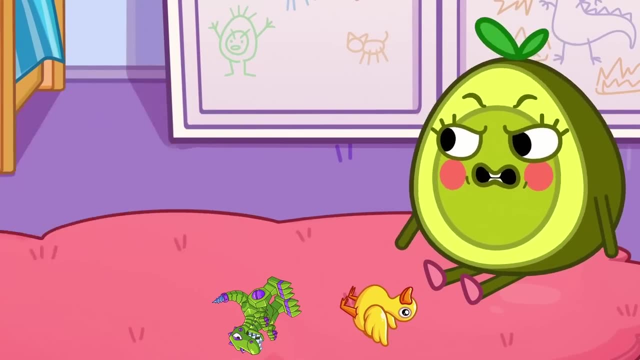 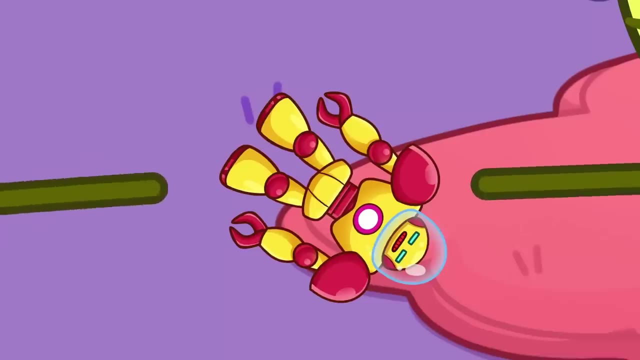 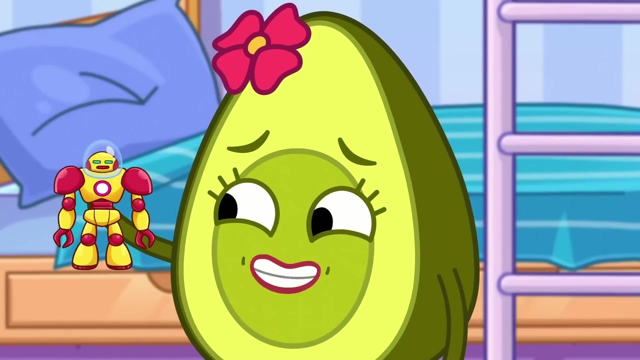 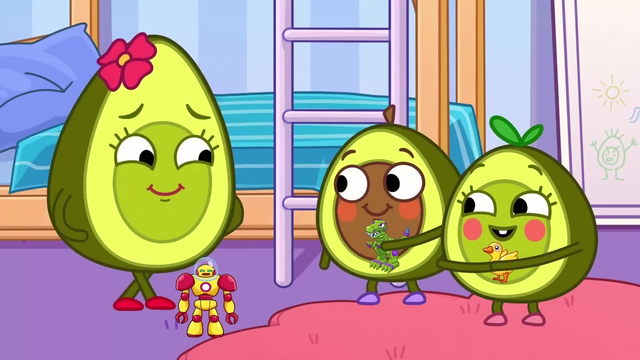 The kids are fighting over a toy. I'll play with the robot. No, Here's your toy. Maybe mommy can help. If you can't decide, I can play with the robot Pit Penny. Go, grab another toy, Let's play. 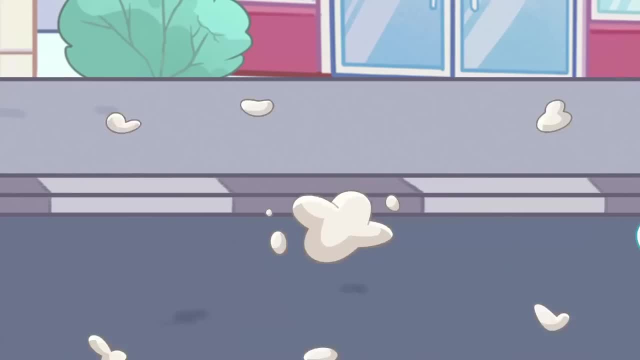 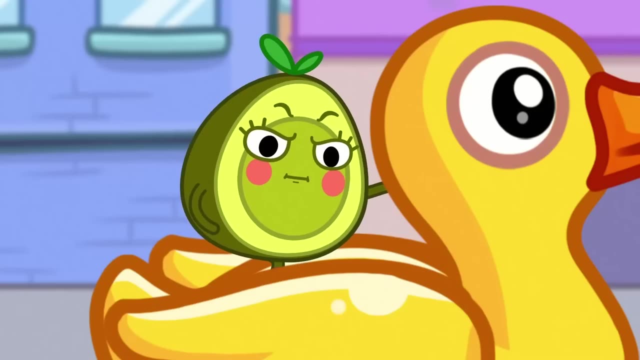 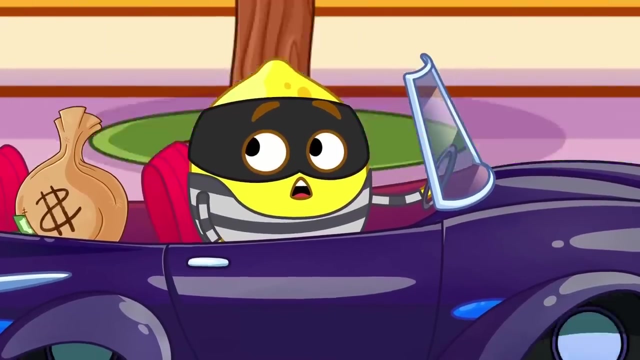 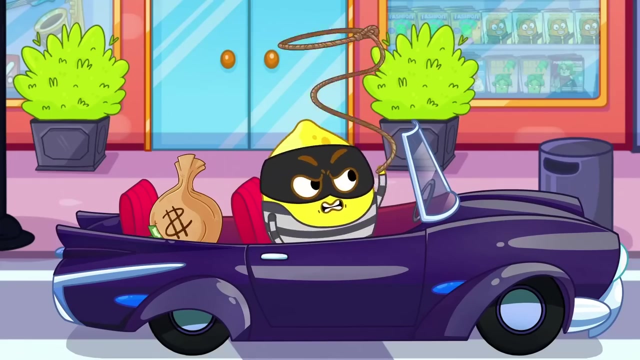 Oh no, Mr Lemon robbed a bank. Penny will stop him. Get him Pit, Penny stop him, And the robot will be a bit of an accident. Penny's been caught, Must be, you know. Take that, Penny's been caught. 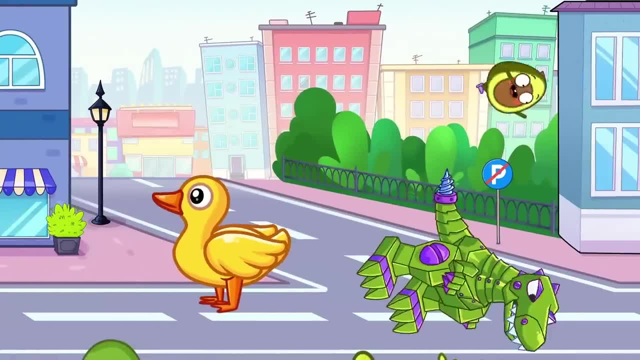 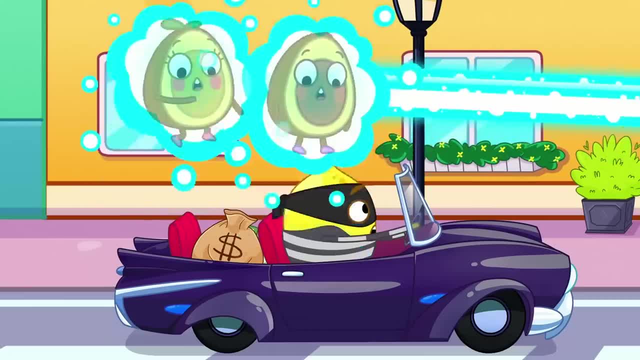 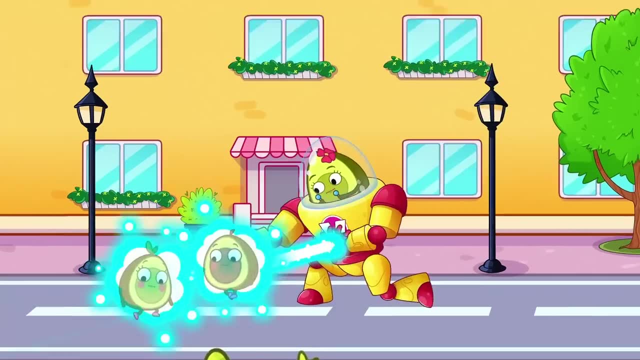 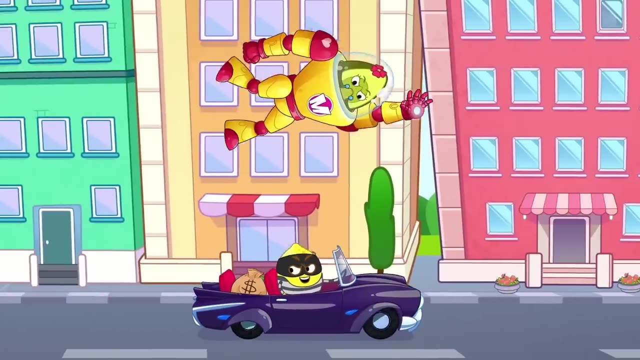 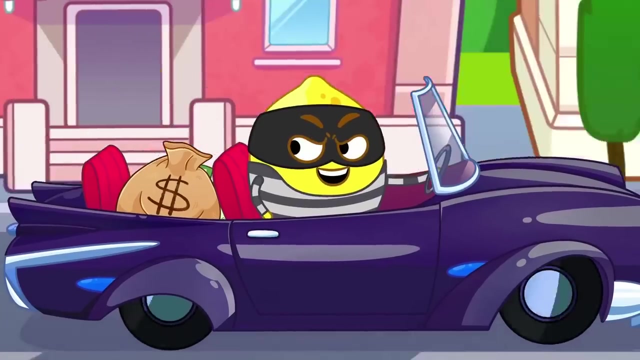 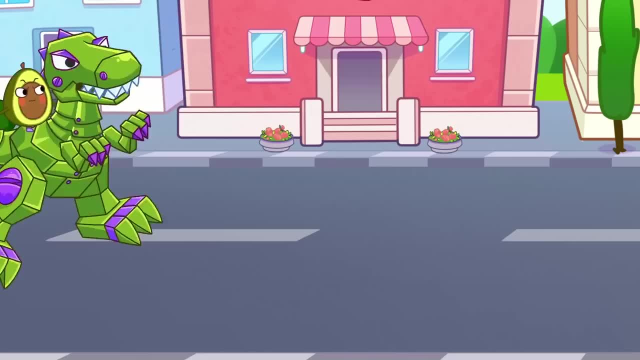 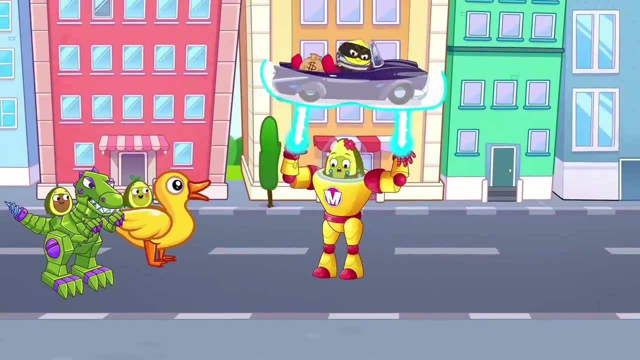 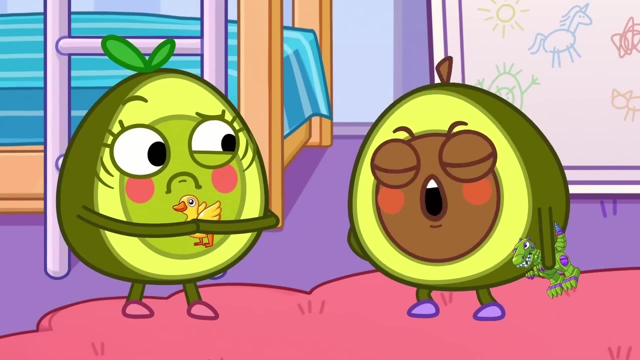 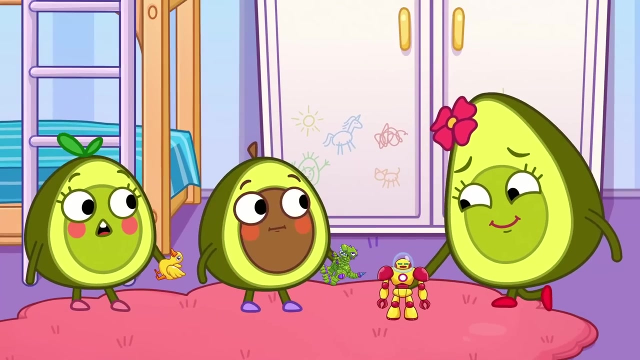 Of course she can. Got you Careful kids, Don't bounce too hard. Look, Mr Lemon is getting away. No, We lost him Because of you. No, It was you. Mommy has an idea. We need to catch him together. 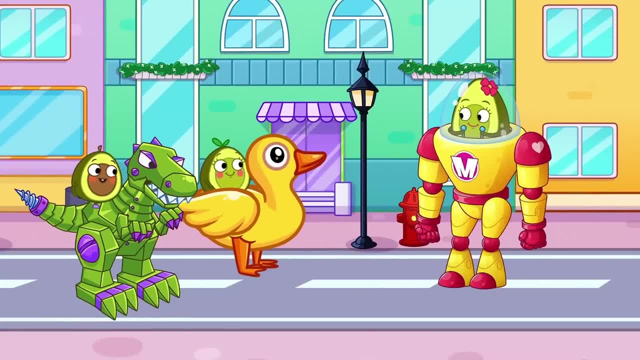 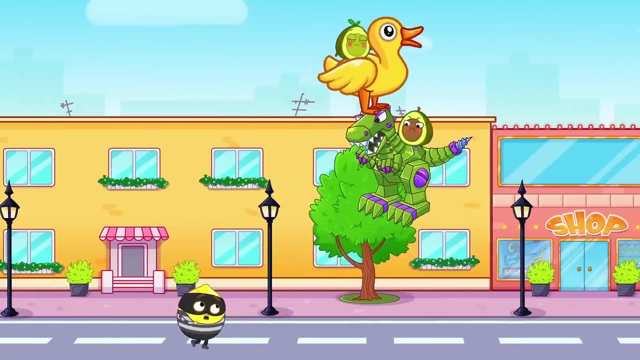 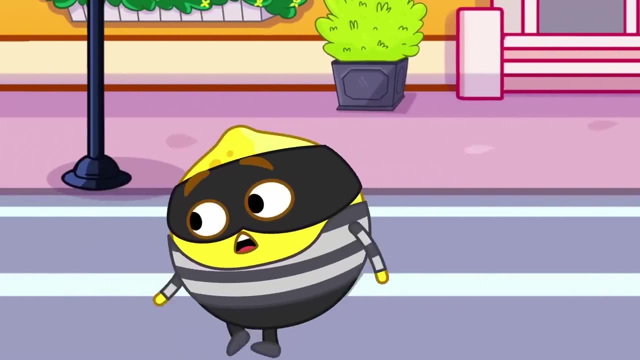 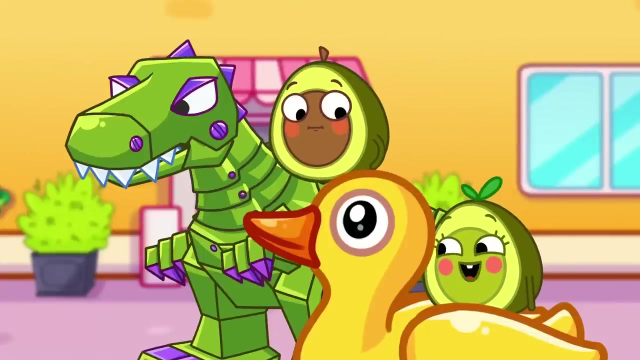 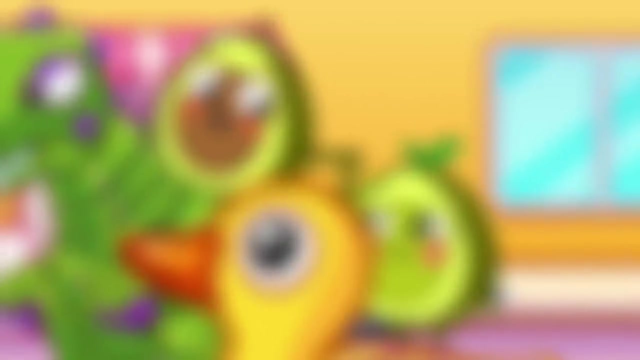 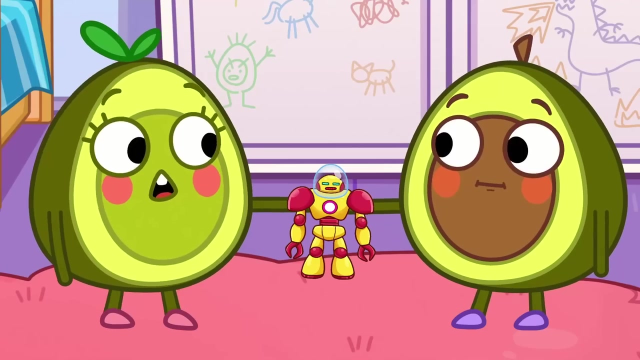 Time for some teamwork. Follow me Up, Hit'em. Penny and Mommy saved the day. Mom, You got him. No, We did it together… Now you can take turns playing with the robot. It's always best to work and play together. 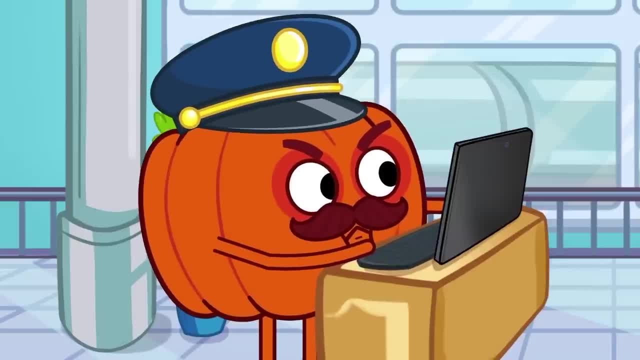 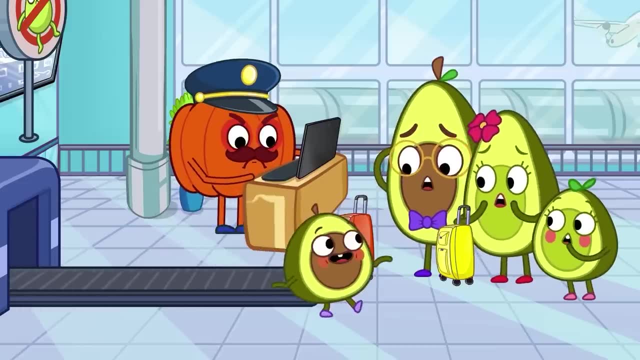 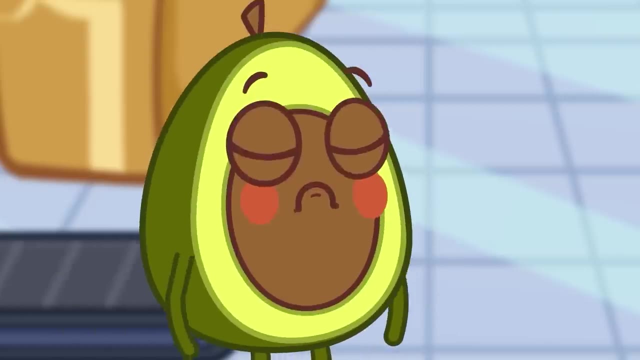 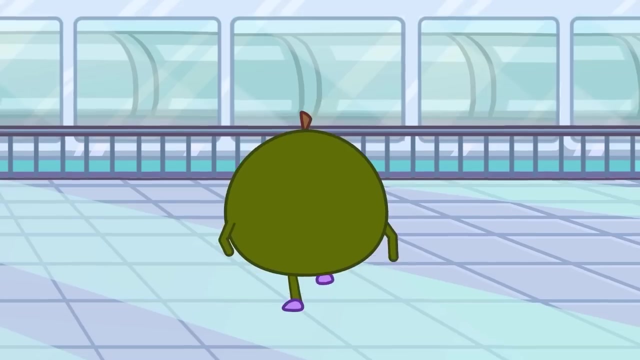 Here comes the luggage. Officer Pumpkin makes sure it's all safe. What did he see? Oh no, It's Pit Pit. You can't get on luggage belt. They can be dangerous, I'm sorry. Uh, wait, Now where's Pit going? 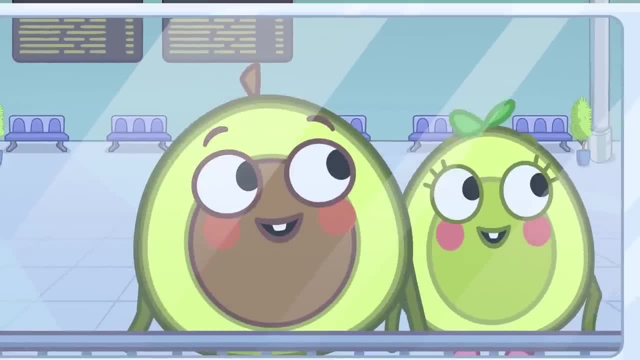 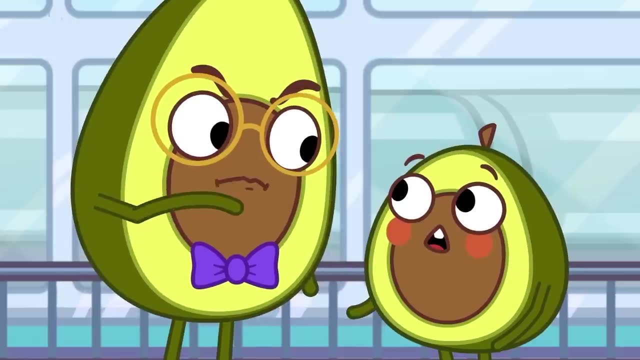 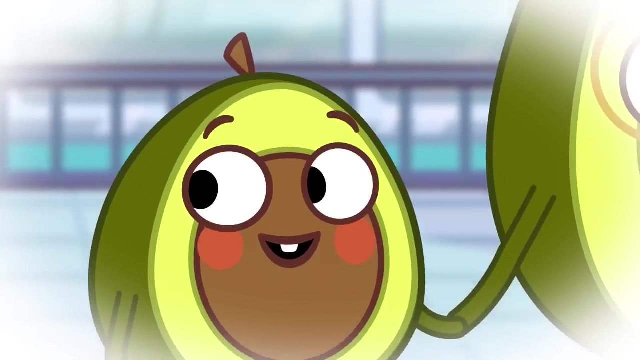 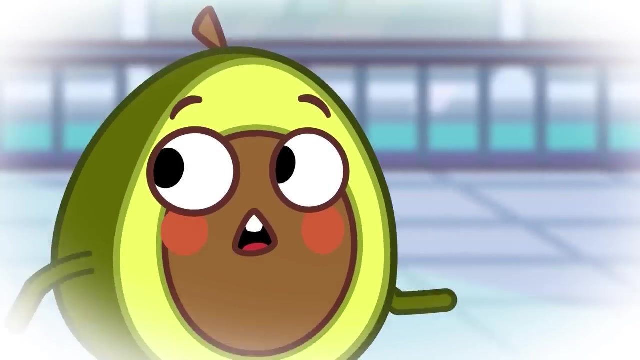 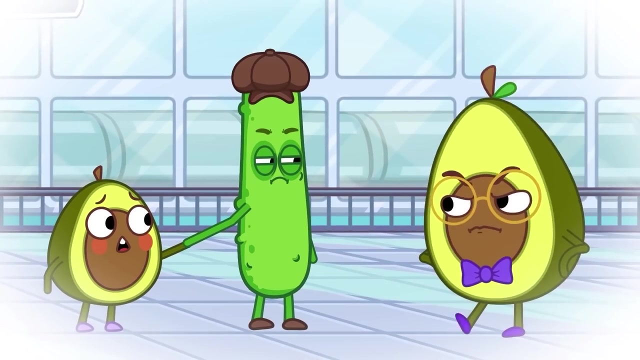 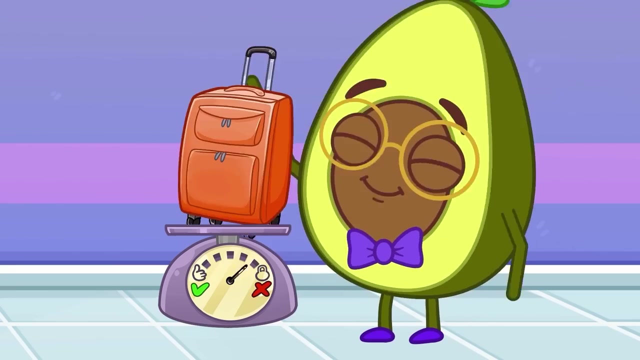 He loves watching the planes take off. Don't run away from us. It's easy to get lost here. Airports can be very crowded. See Pit lost Daddy. That's not Daddy. Now let's weigh the luggage, Yay. 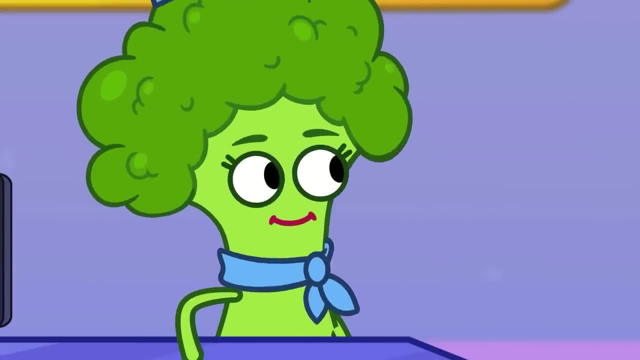 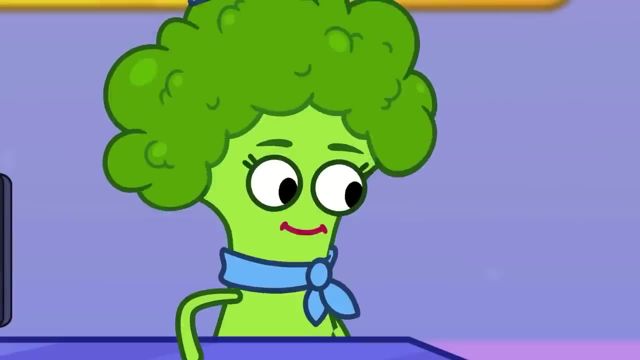 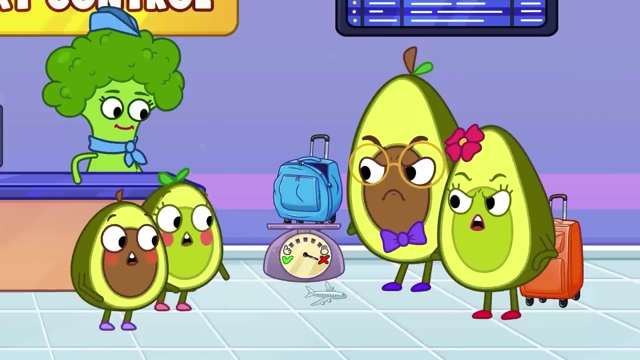 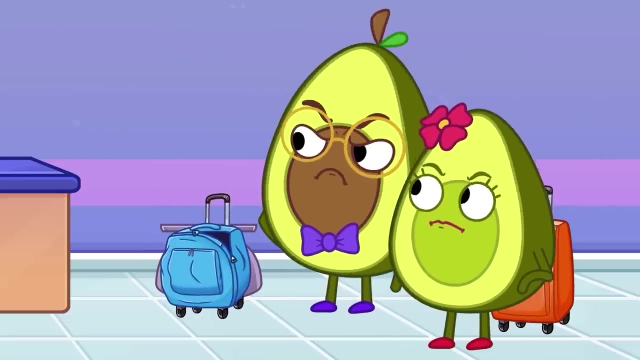 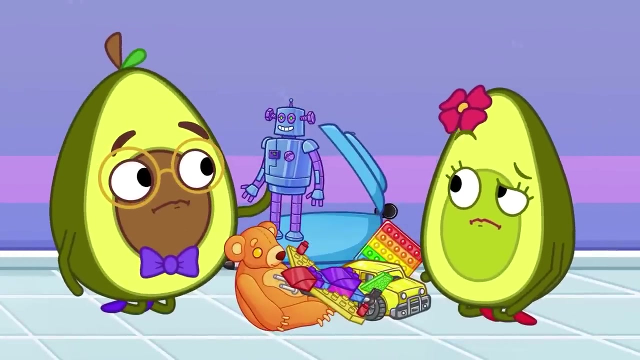 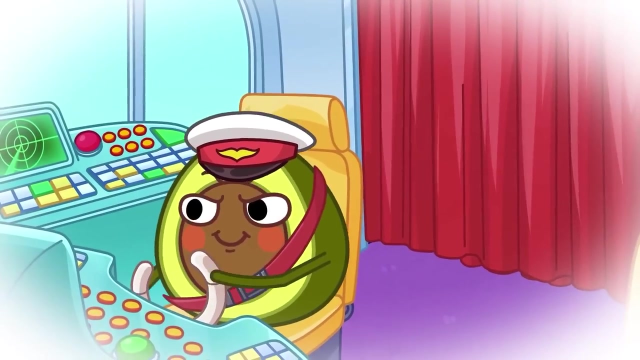 It's the perfect weight. Now let's weigh Pit's suitcase. It's too heavy. He packed too many toys. Aww, Aww, Pit, you've taken too much stuff. Pit thinks the plane can carry all his toys, Uh-oh. 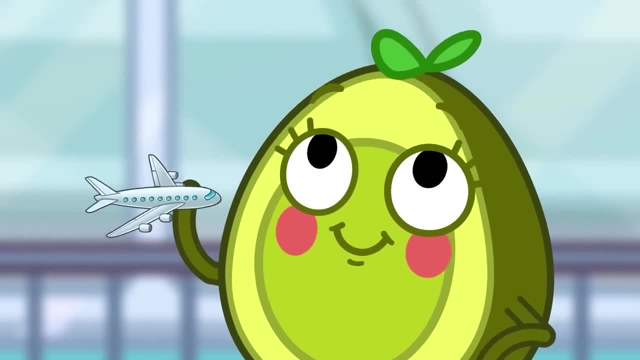 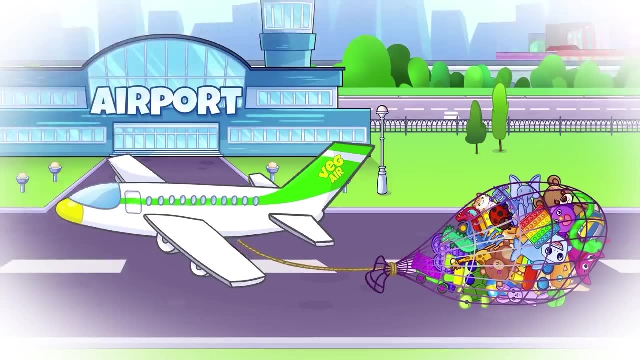 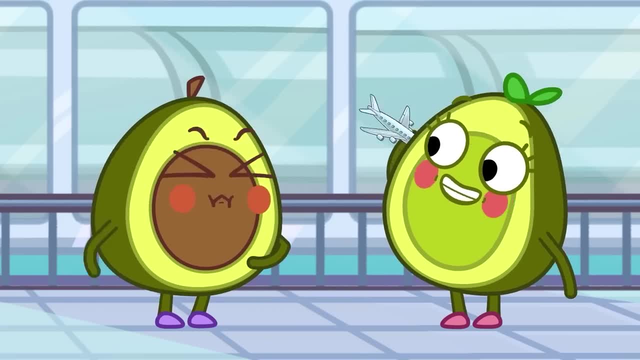 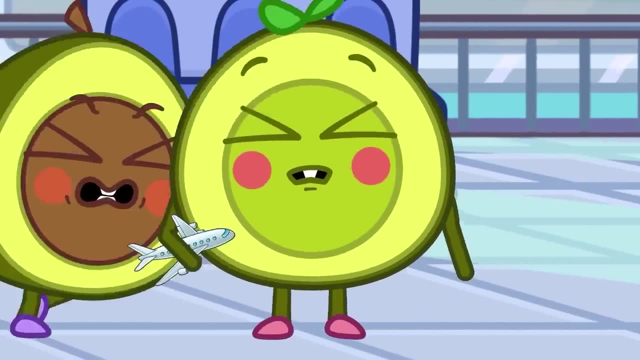 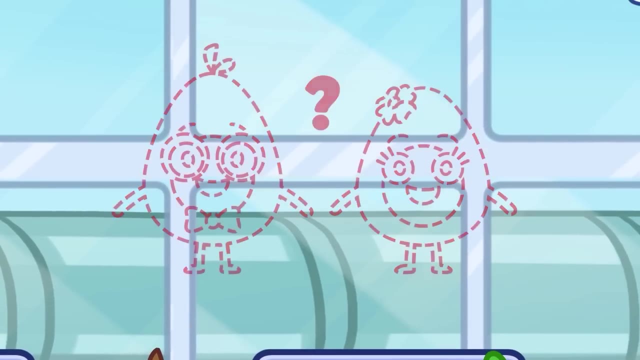 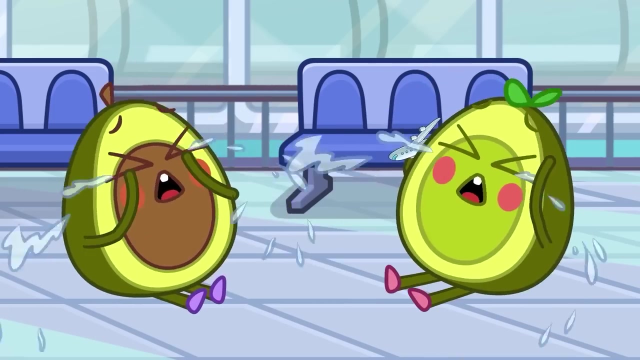 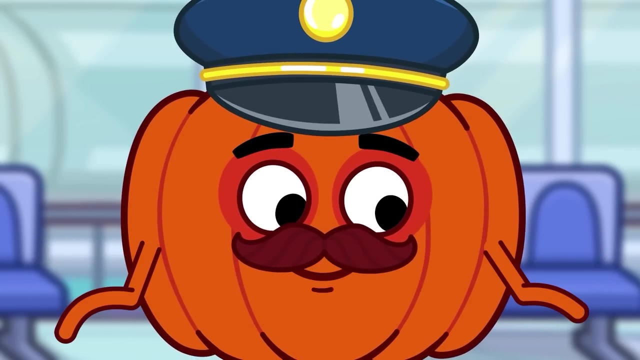 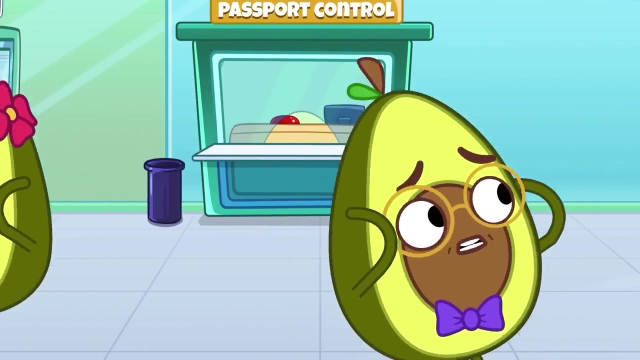 If the plane is too heavy, it can't fly. encounters his stepdad. Oh no, They left without us. Maybe Officer Pumpkin can help. Kids, Don't cry. I'll take it to your parents See how worried Mommy and Daddy are. 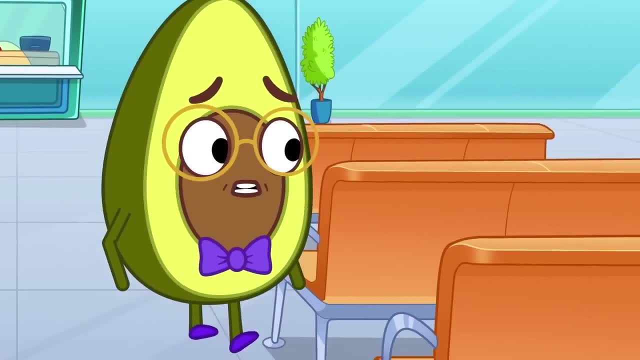 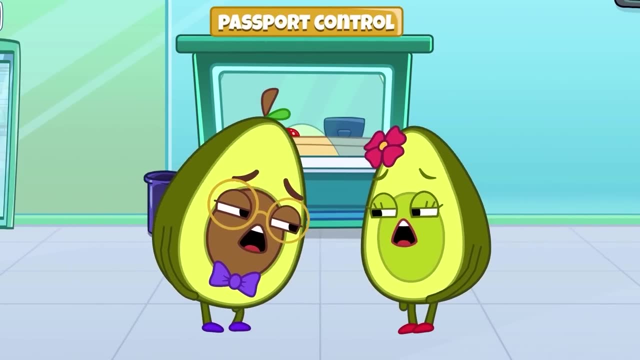 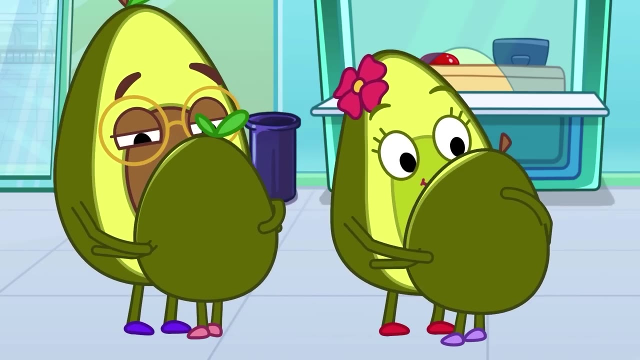 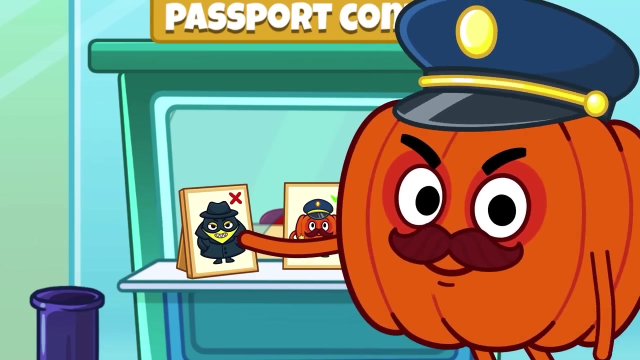 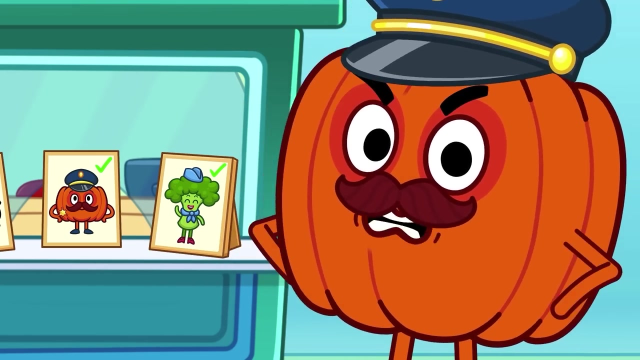 Pit Penny. They're looking everywhere for Pit and Penny. Pit and Penny are safe. Thank you, Officer Pumpkin. Remember kids don't talk to strangers at the airport. If lost, ask a police officer or flight attendant for help. 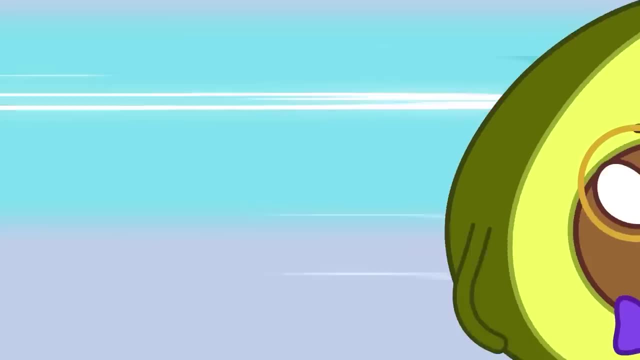 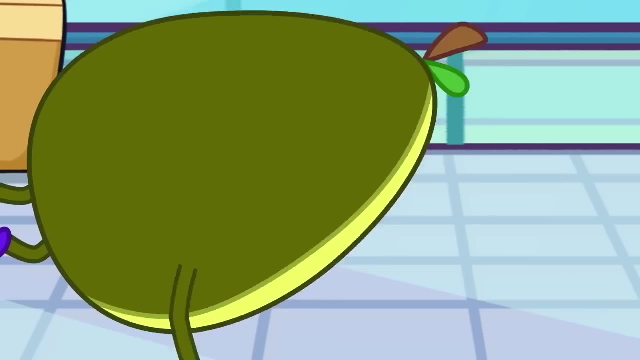 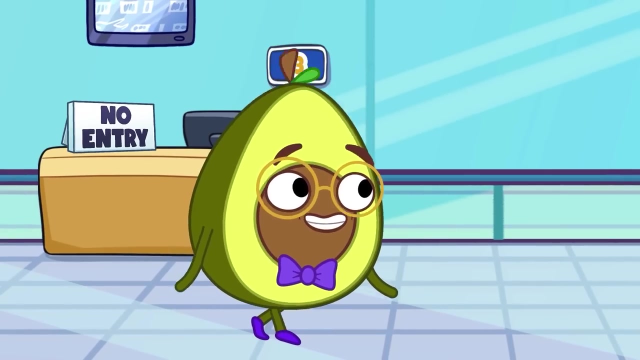 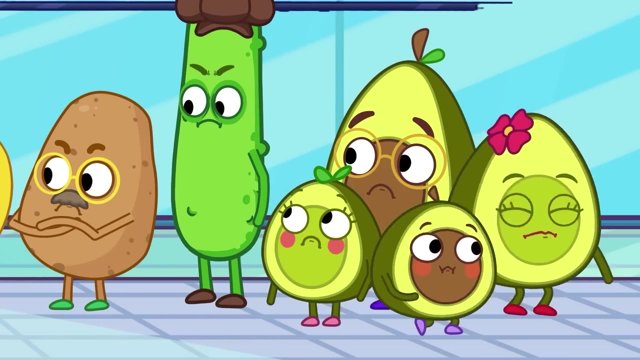 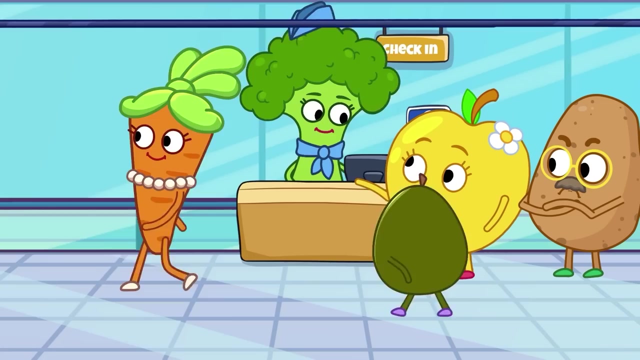 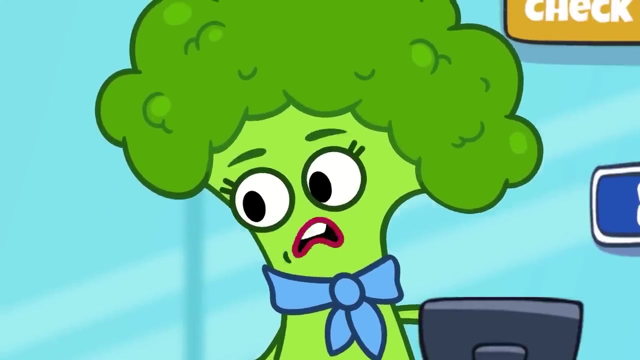 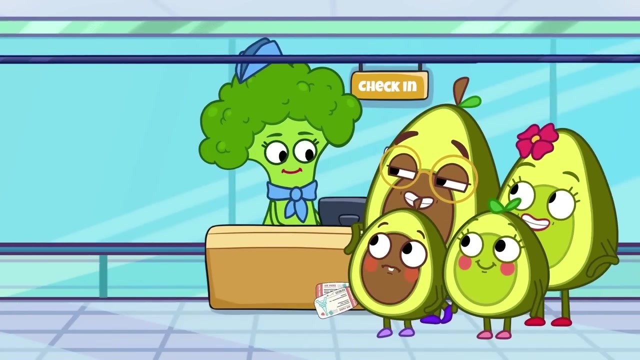 Hurry, The plane leaves soon. No Wait, It's okay, Daddy, There's another line. Pit doesn't want to wait in line. It's important to stay in line. You need to wait your turn, Pit. Now the flight attendant can help you. 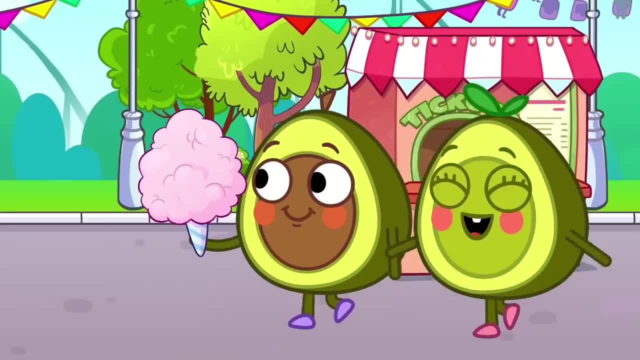 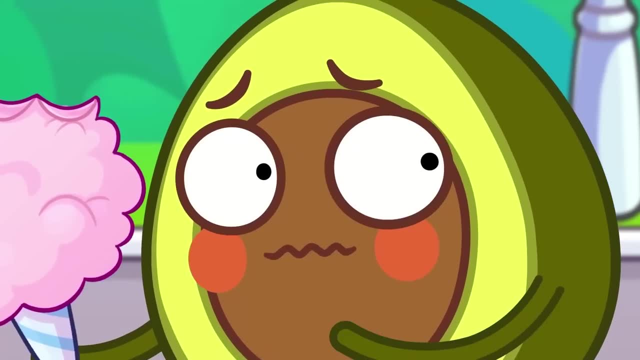 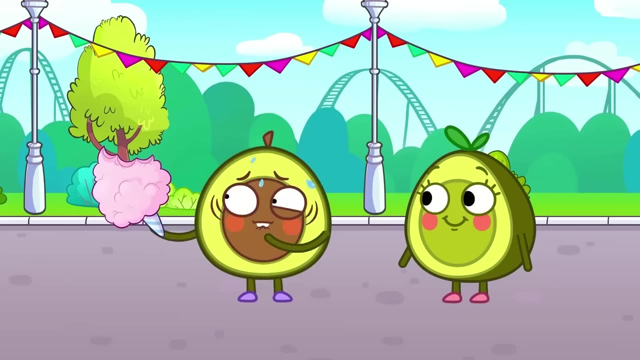 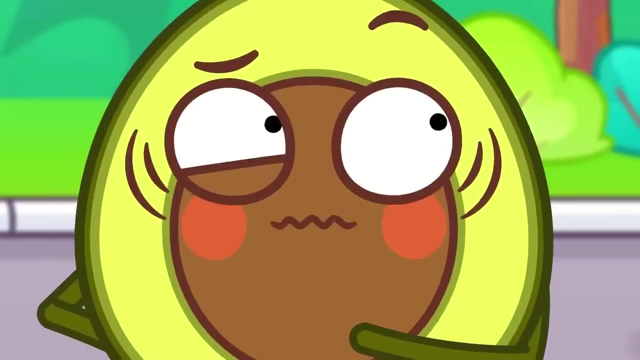 Have a fun trip. Pit and Penny are at the fair, But Pit's tummy feels yucky. Sorry Pit, but that potty is out of service. What should Pit do? No, Pit, Don't go in that one. 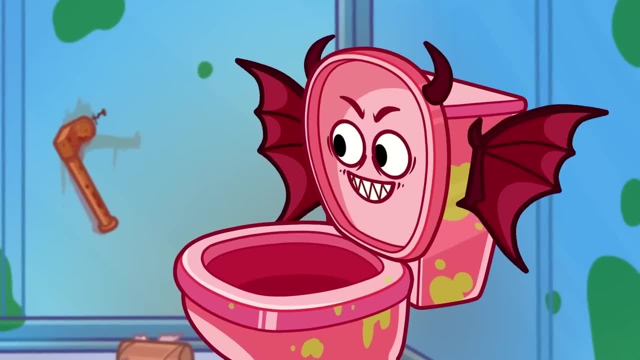 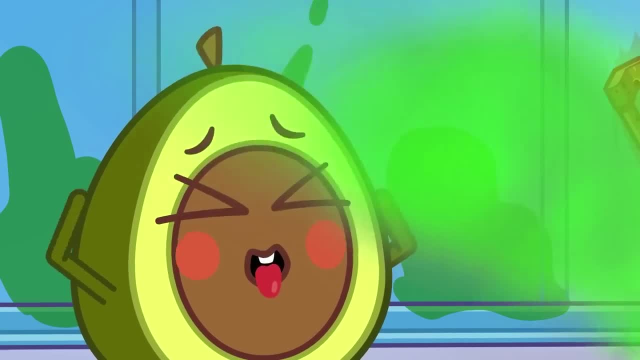 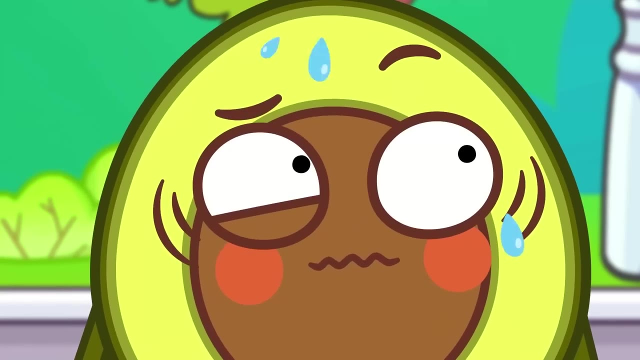 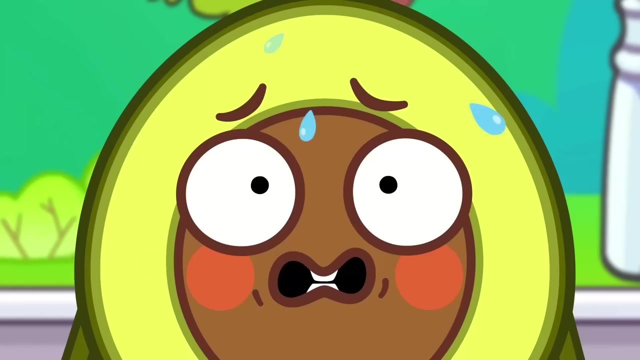 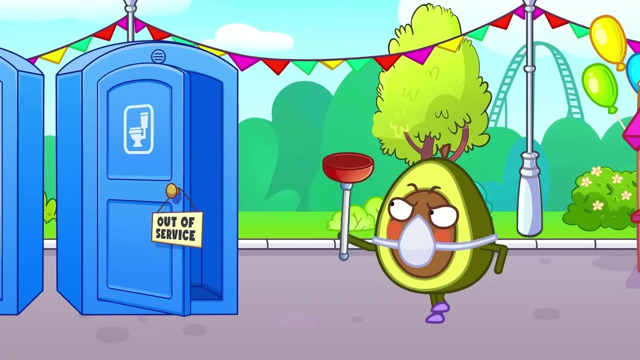 Ew, That toilet looks scary And it smells really bad too- Pee-yew. But the line for the other potty is very long. Now what will Pit do? Pit has a plan And a plunger. Go get him Pit. 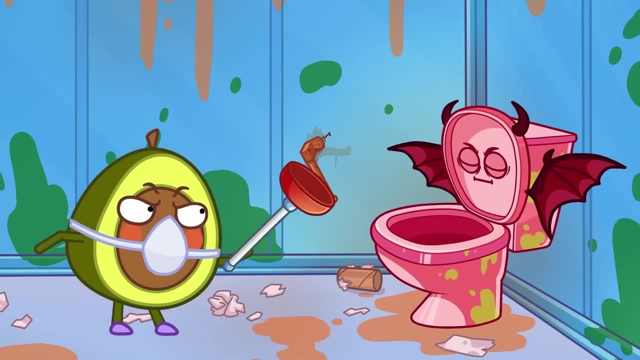 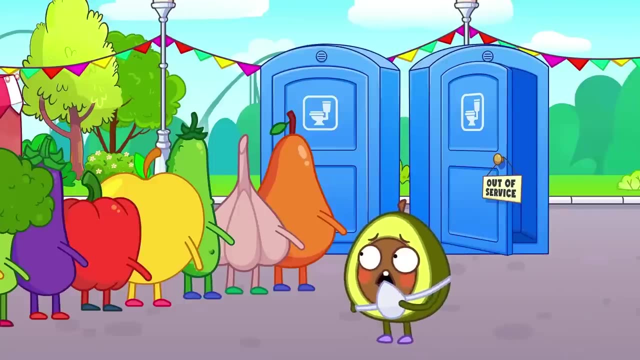 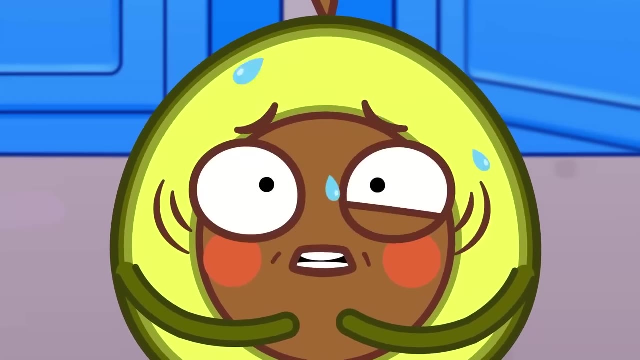 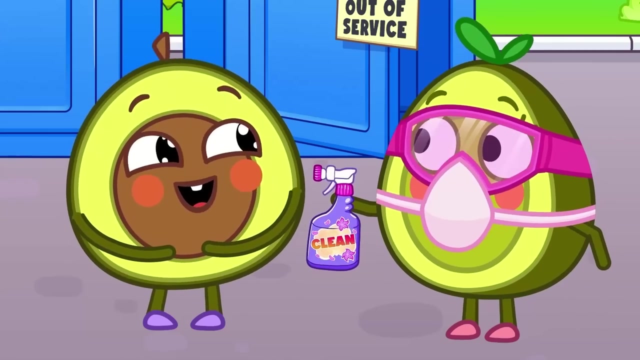 But be careful, That nasty toilet is up to something. Now the line is even longer. Penny's here to help And she brought cleaning spray. Pee-yew, Pee-yew, Pee-yew, Pee-yew, Pee-yew. 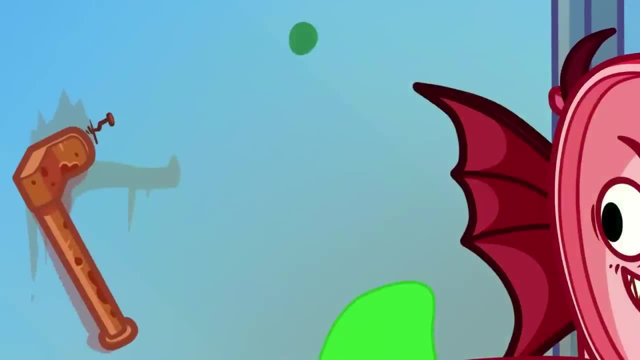 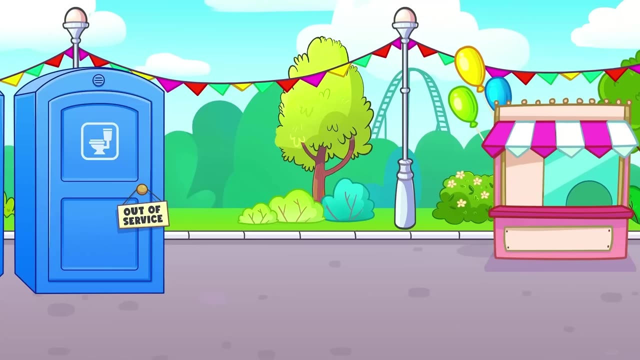 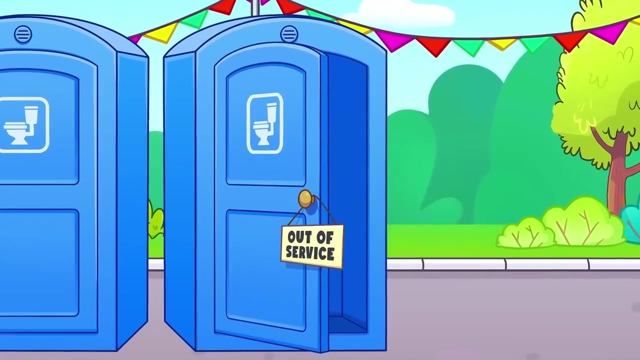 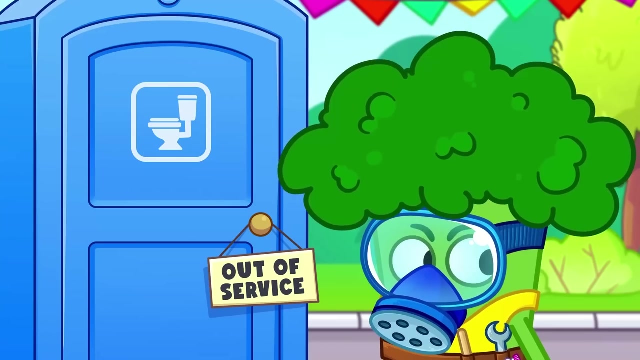 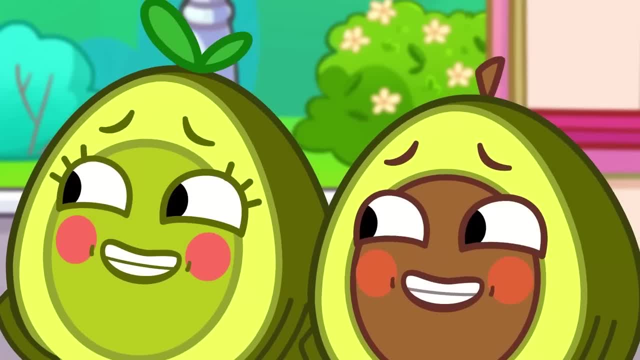 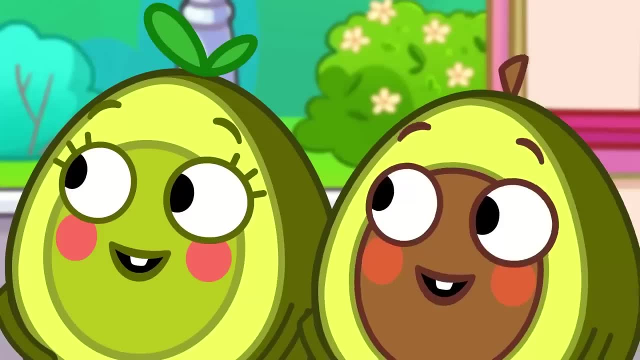 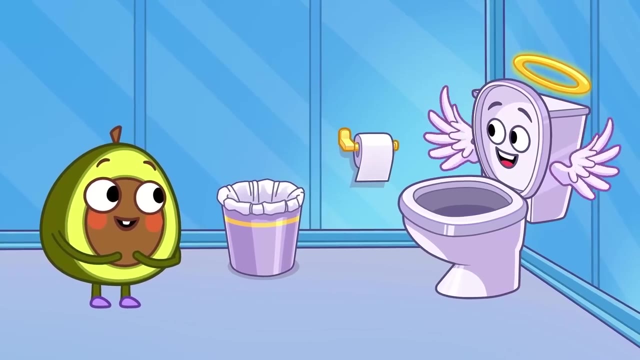 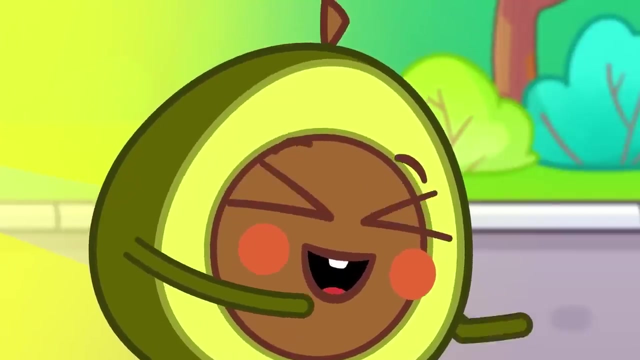 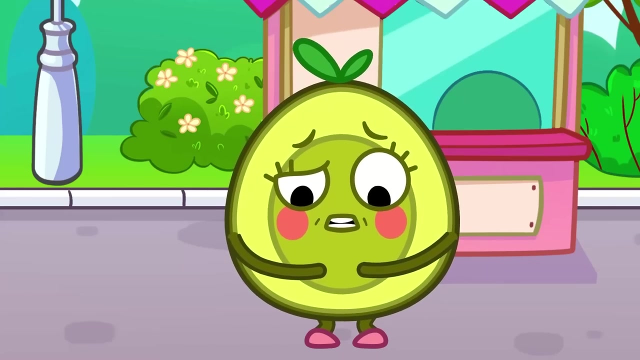 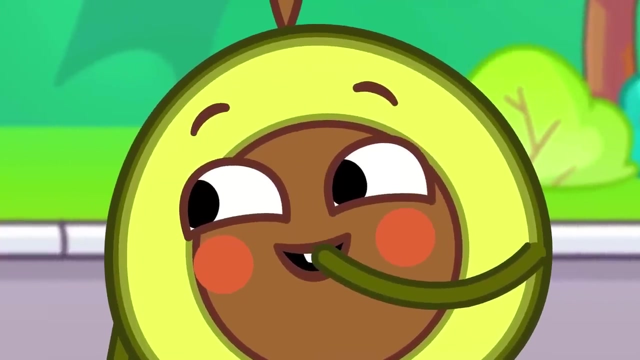 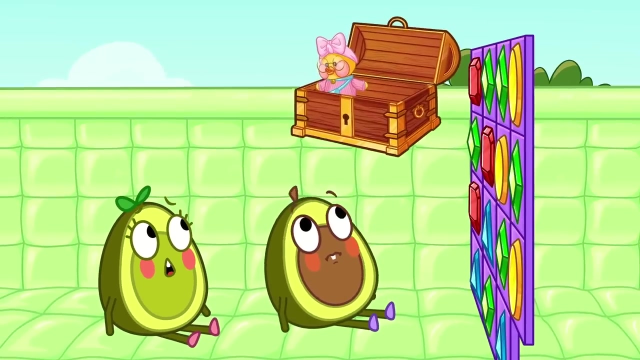 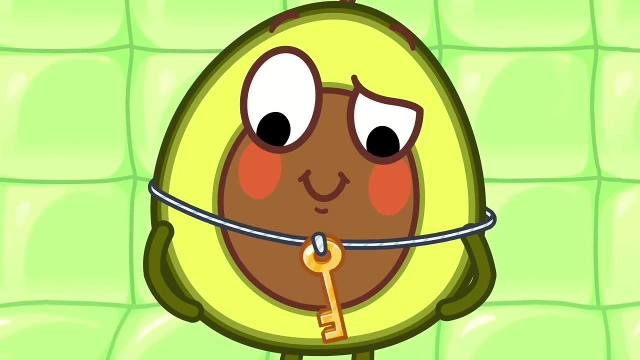 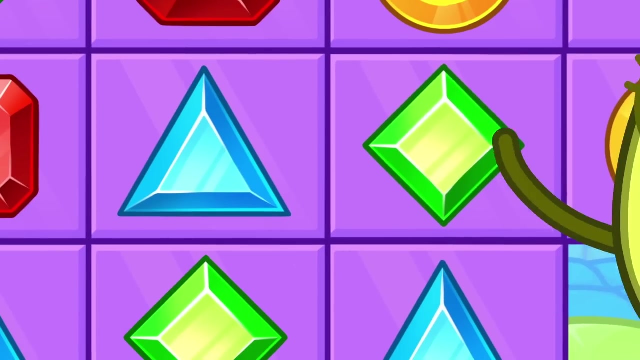 a troublemaking toilet. all done, it can use the potty. what a relief. thank you, janitor. look out, it's Penny's turn now. hidden penny want to watch Lala fan fan duck, but she has a challenge for them. first challenge: get three shapes in a row. 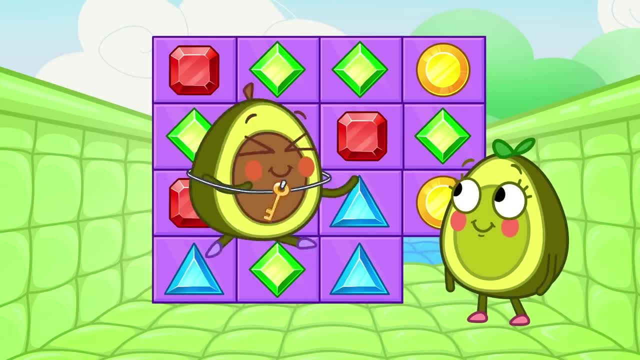 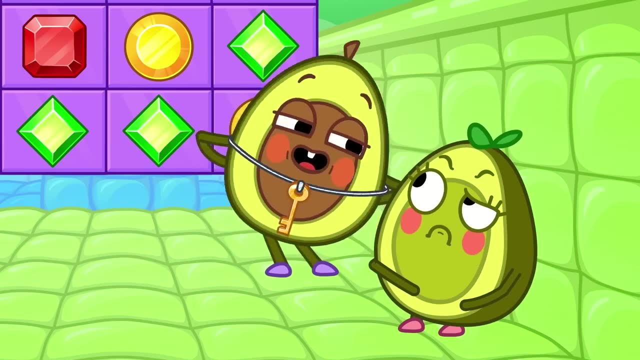 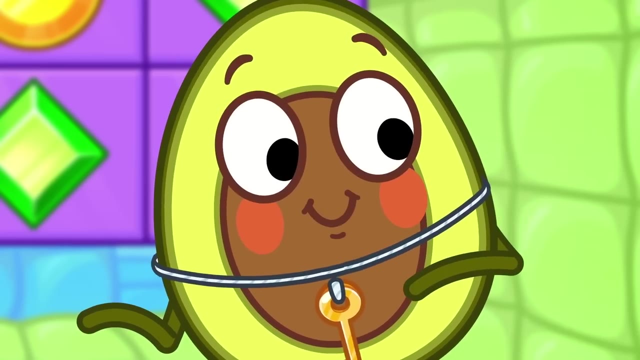 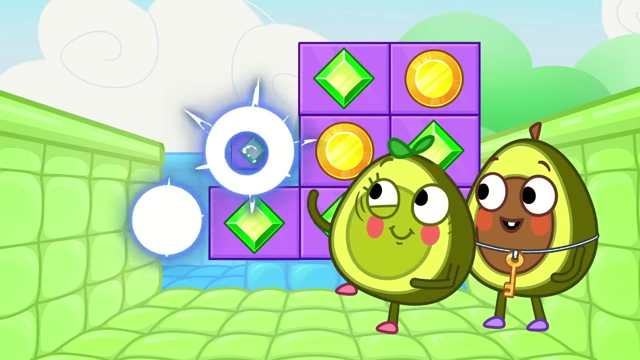 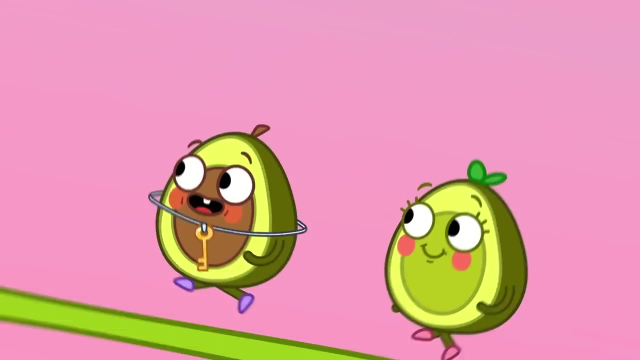 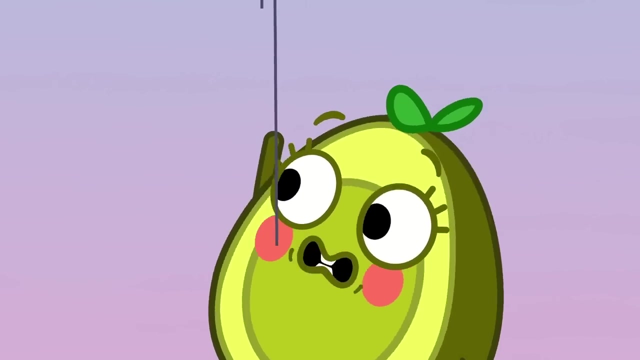 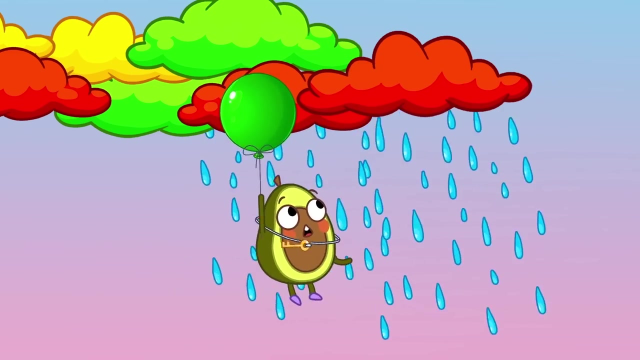 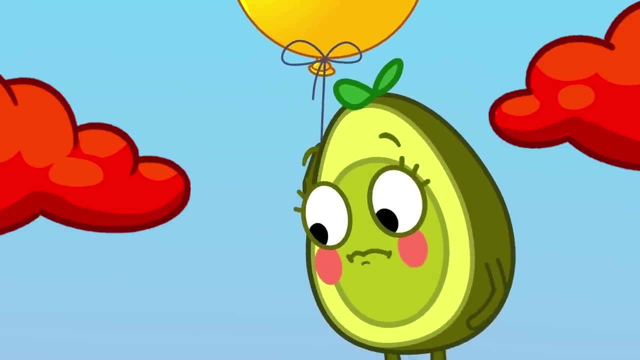 I'm sorry, let's do it together. you can each take turns. quick, grab a balloon now. what should they do? my color is yellow. your turn pit, oops, wrong color. what should he do? penny, look at the color of your balloon. I only need my favorite color. it's green. 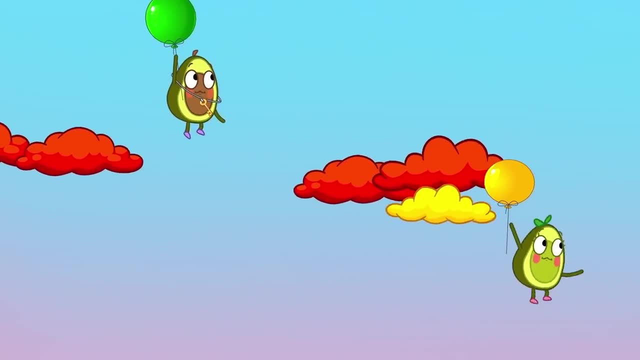 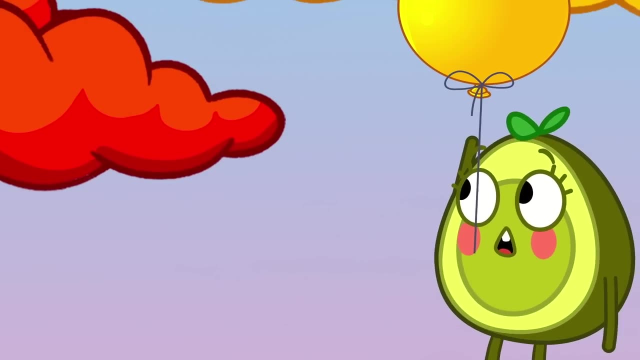 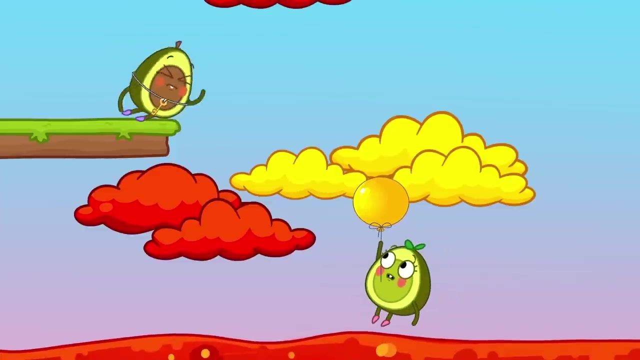 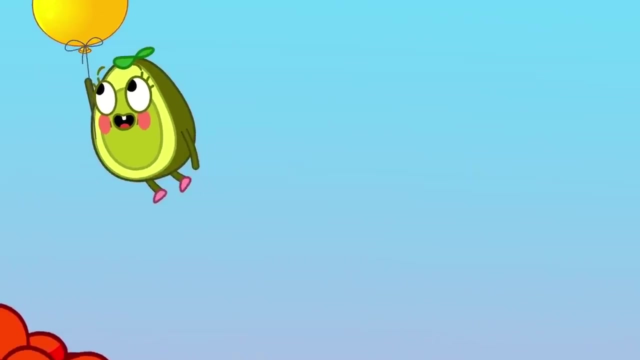 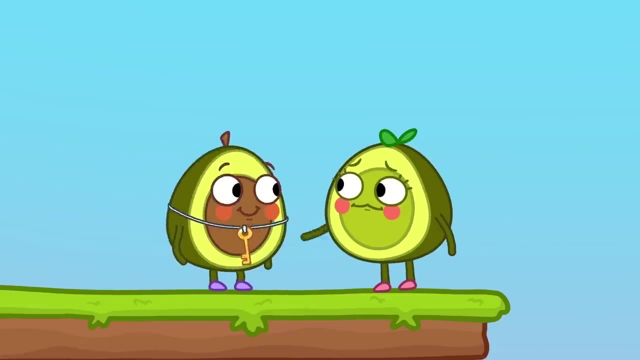 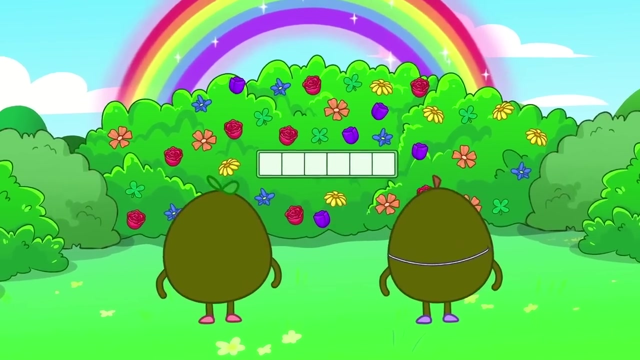 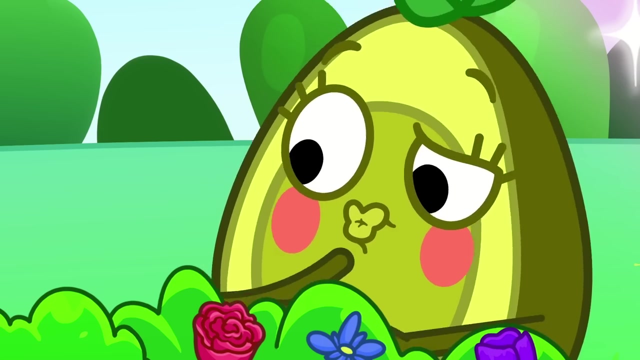 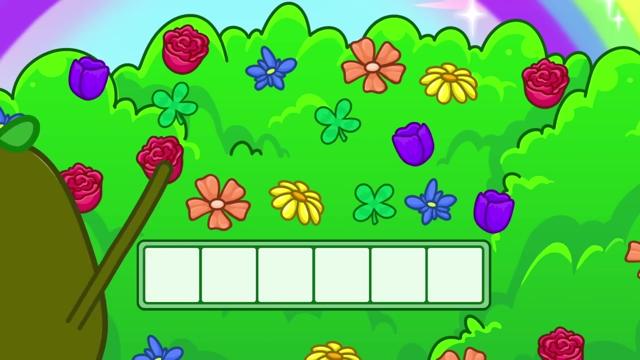 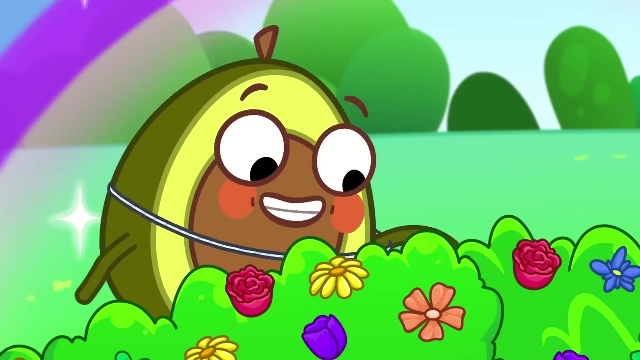 jump on the platform. penny's stuck and Lava is coming. I can help you. it's my mission. well done, Benny. we need to hurry. it's another puzzle. penny knows what to do. we need the same colors: red, blue, blue, blue, red, blue, blue, blue, orange, orange. 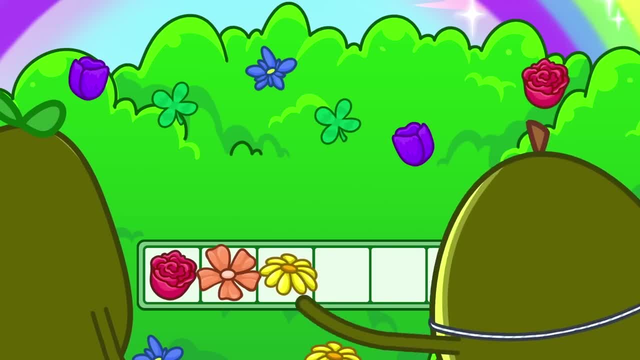 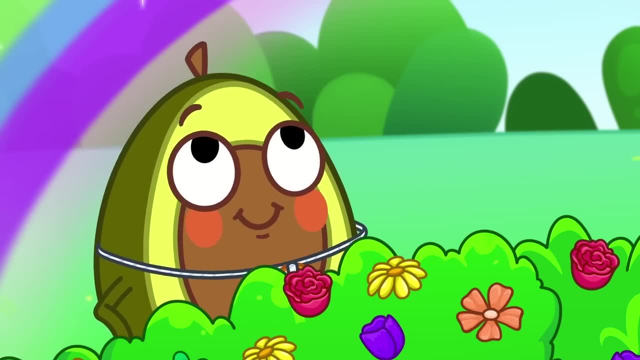 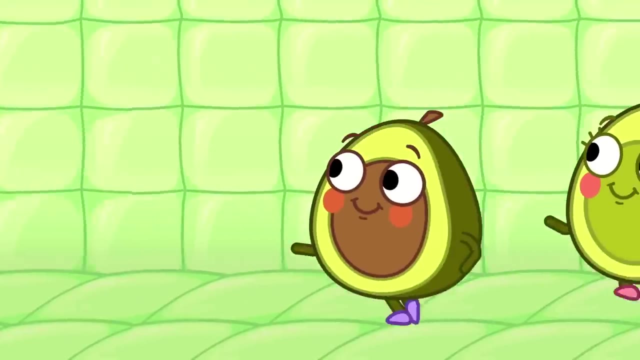 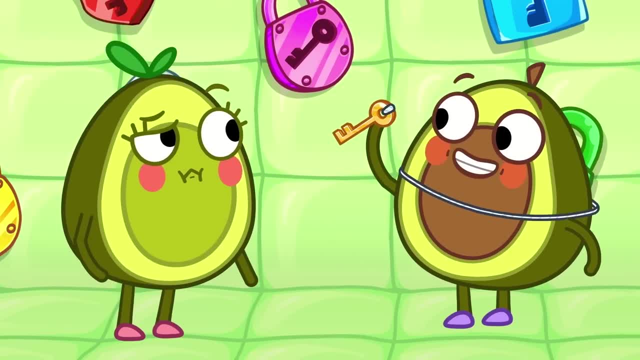 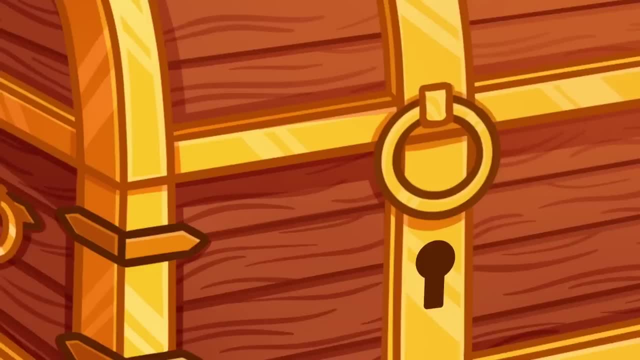 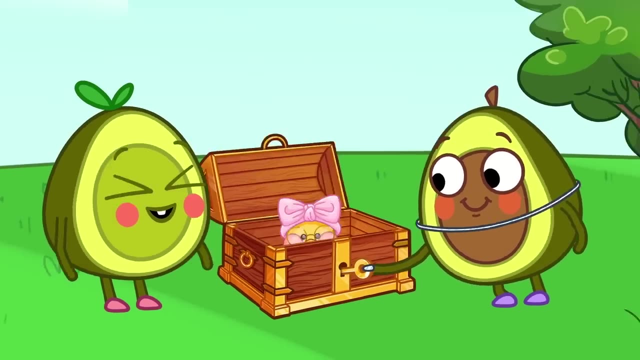 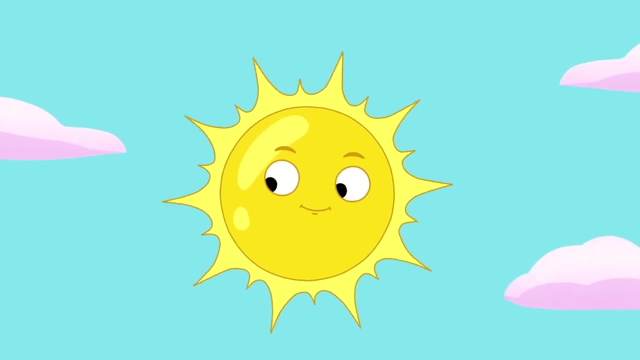 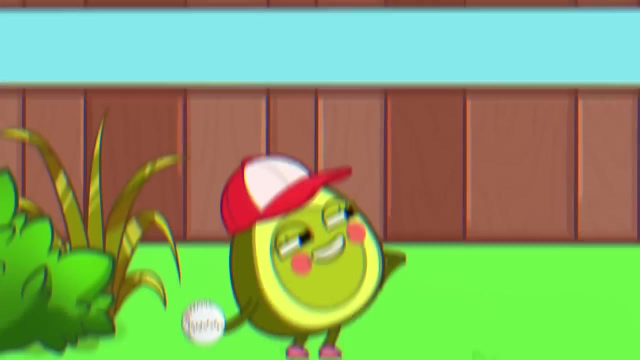 a box, a box, a box. We need the same shape. You did it And here's your prize. It's Lala Fan Fan Duck. We did it. It's a hot sunny day. Maybe it's too hot. The heat's making Penny tired. 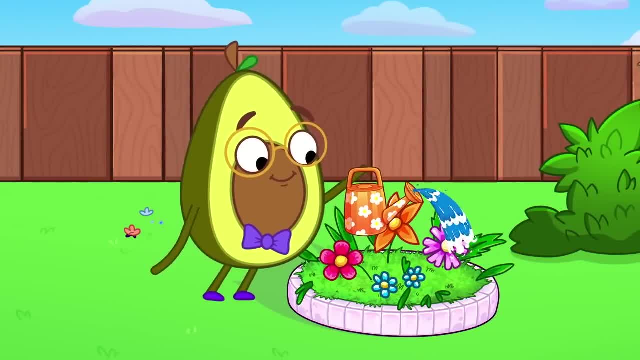 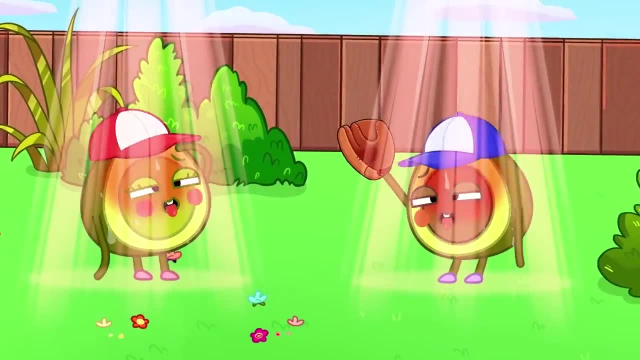 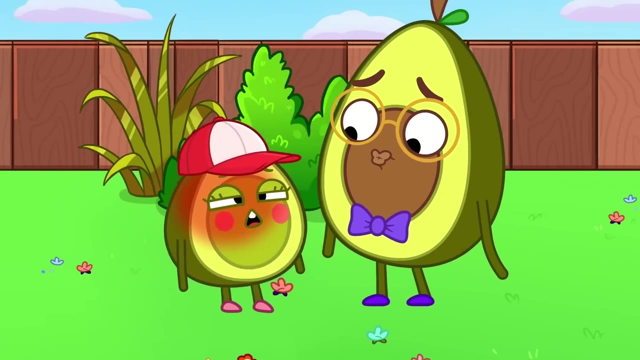 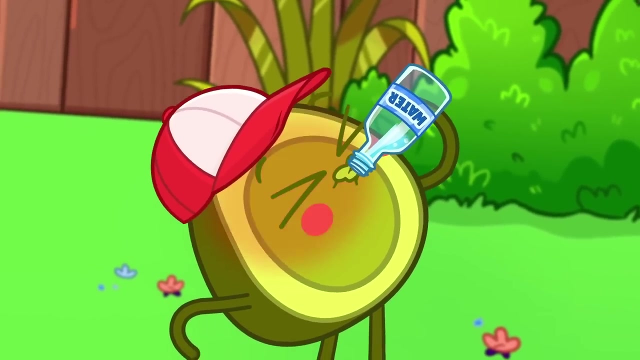 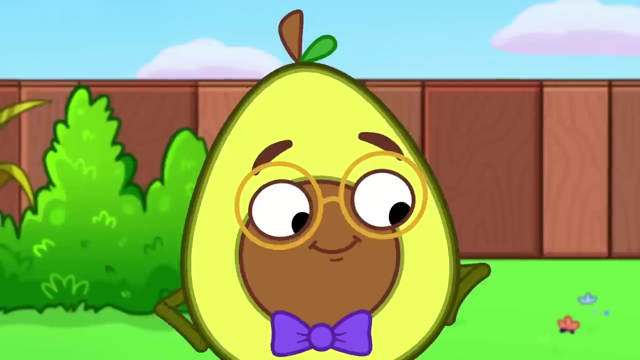 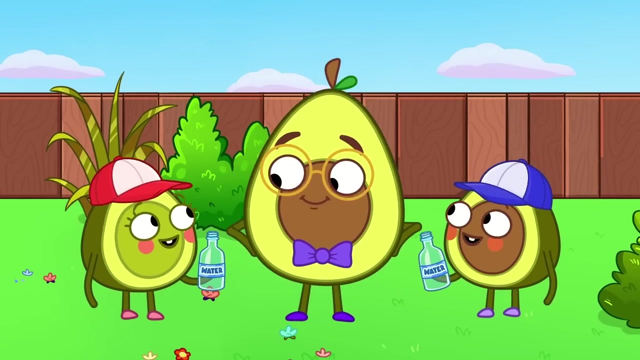 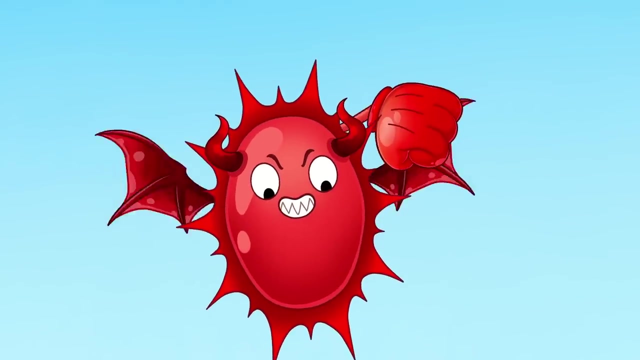 Oh, and Pit's tired too. Pit and Penny need help. What should Daddy do? Aha, Drink some water. What does drinking water do? It'll save you from overheating And then you can keep on playing. The sun is really angry right now. 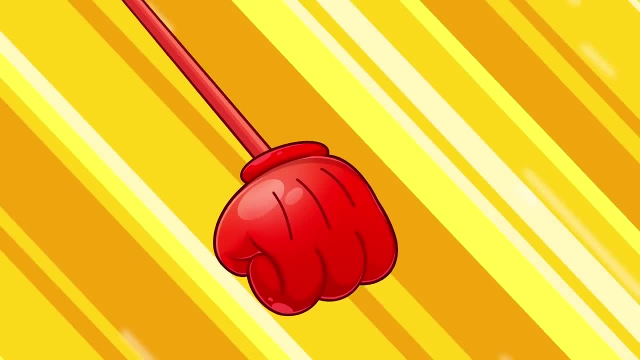 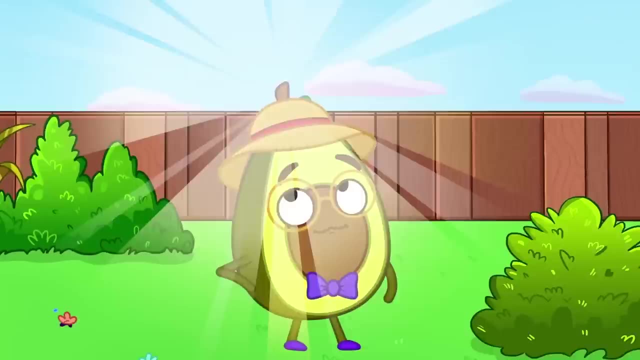 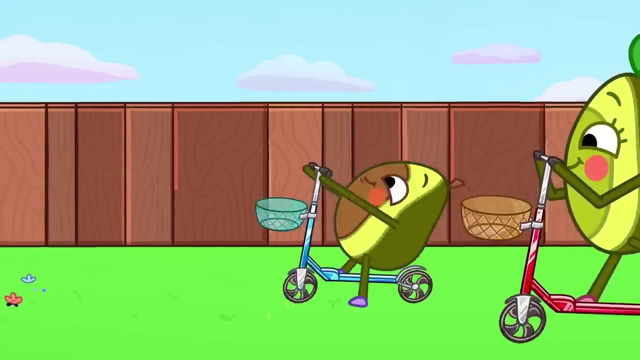 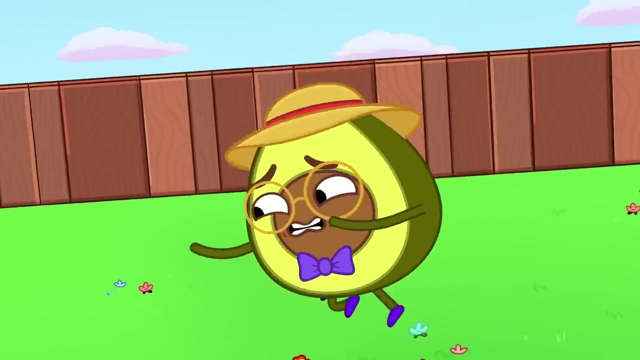 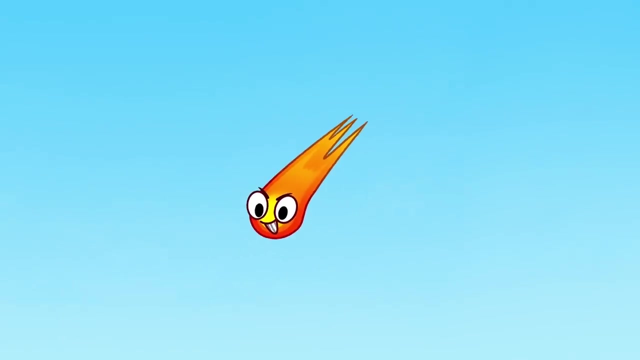 Watch out, Daddy. Daddy's not worried, A hat will protect him. Ah, But what about Pit and Penny? Hahahahaha, Hahahahaha, Ah, Ah, Ah, Ah, Ah, Ah. But what do hats do? 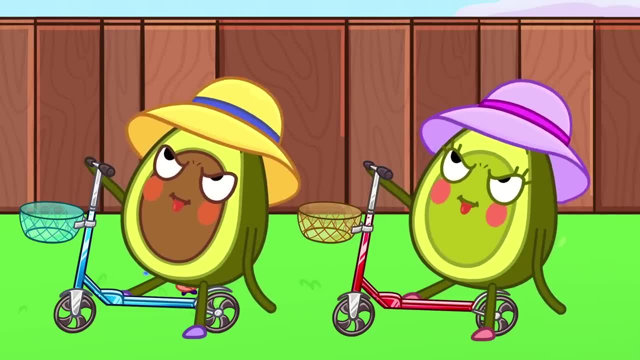 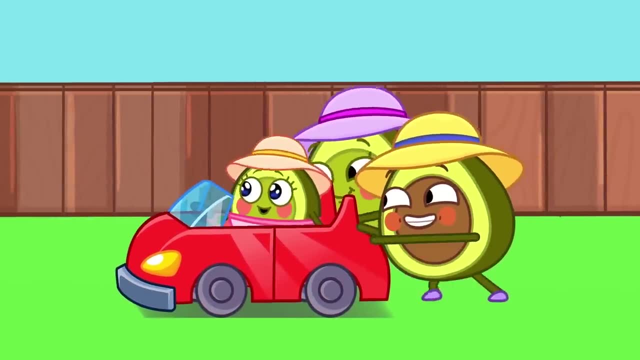 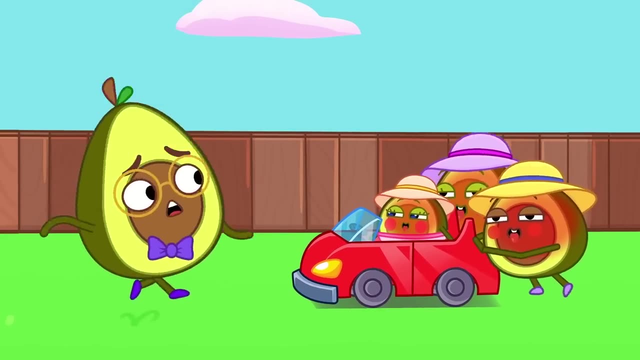 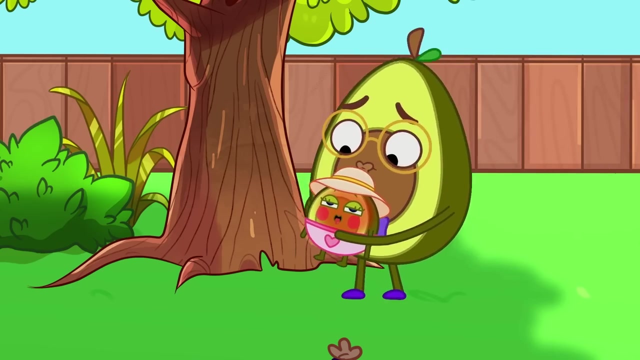 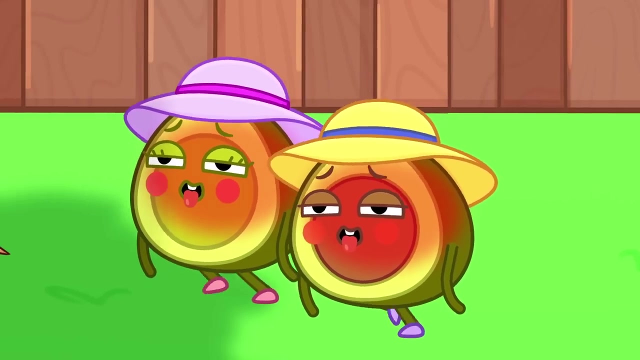 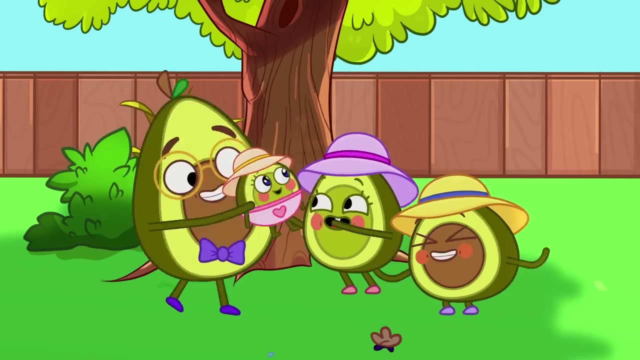 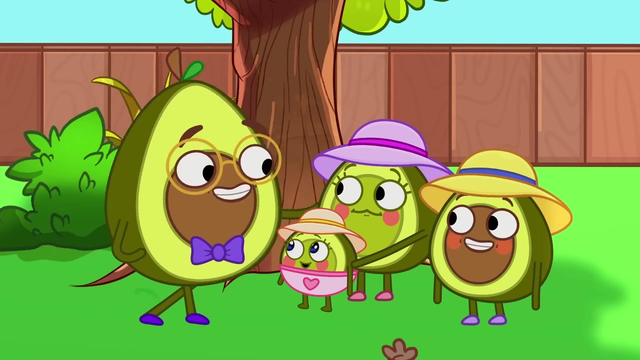 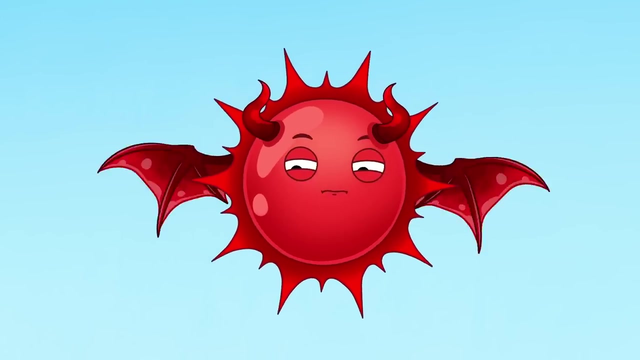 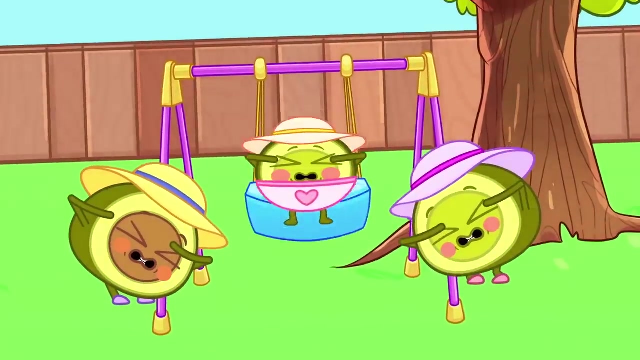 Hats save you from a sunstroke. Now it's gotten really hot outside. Ah, some cool shade will help. Ah, Stay in the shade so you don't overheat. Oh no, The sun is back. Ah, Quick, find some shade. 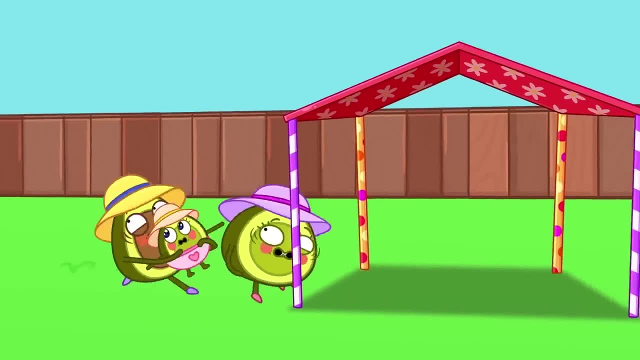 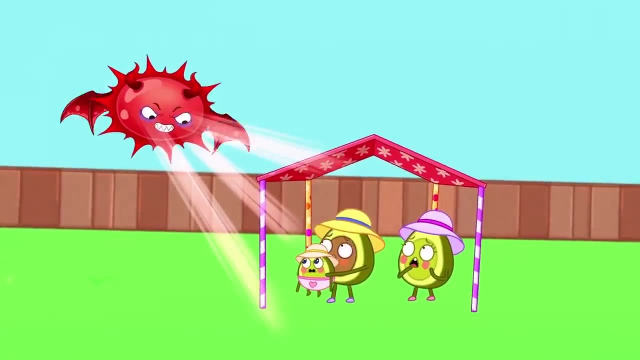 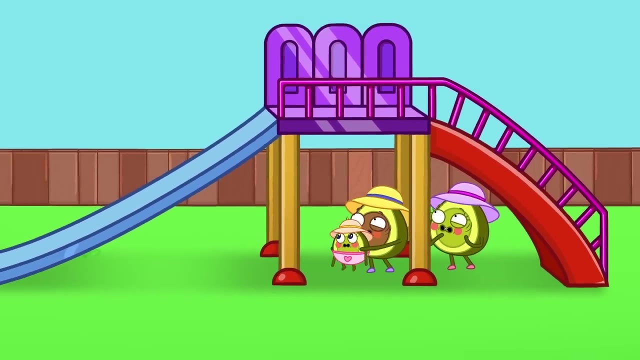 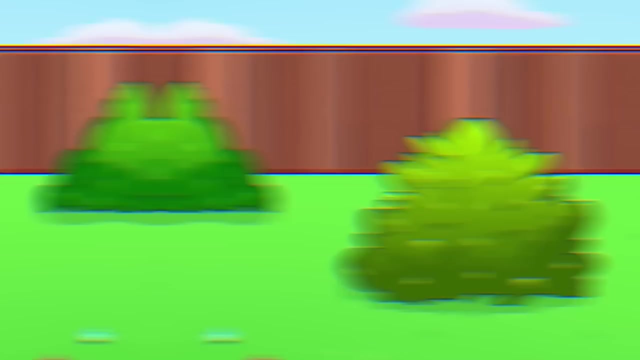 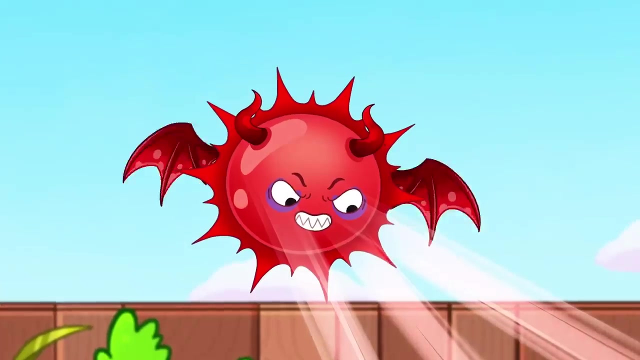 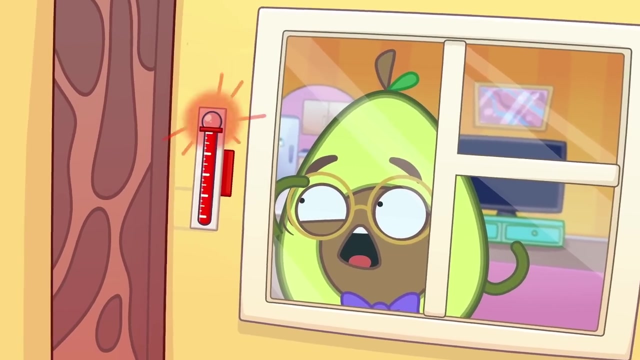 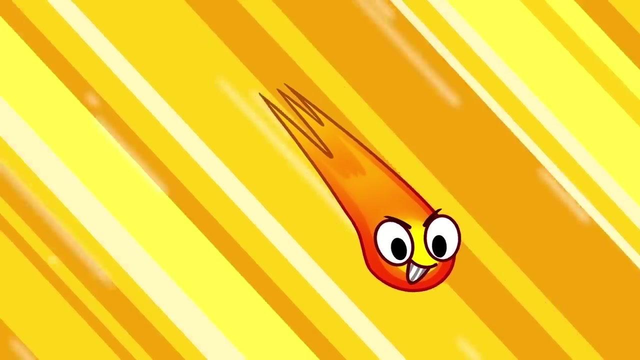 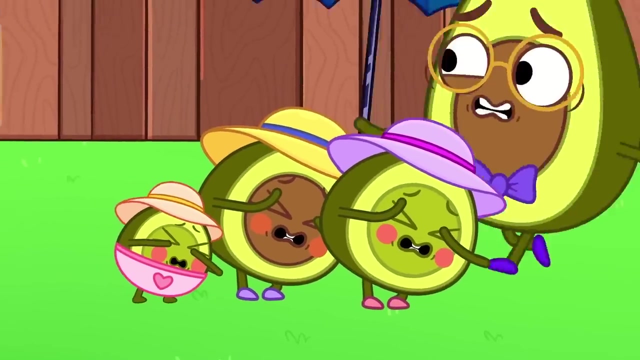 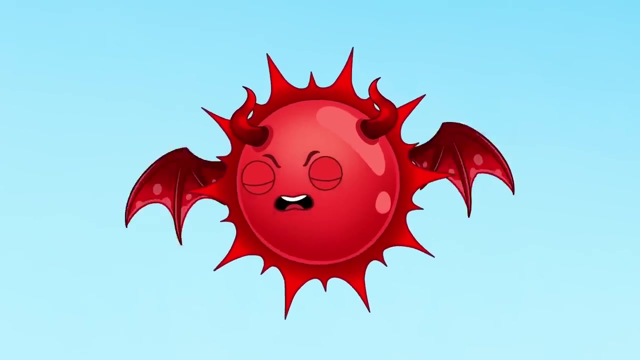 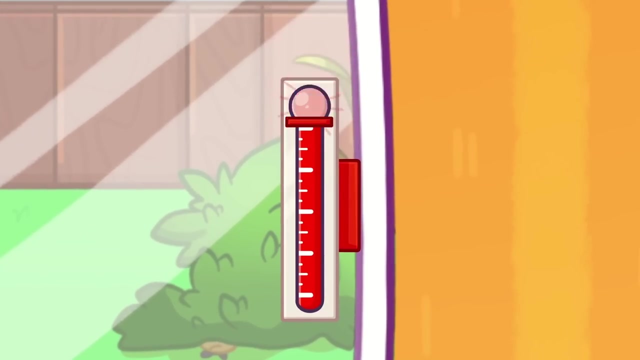 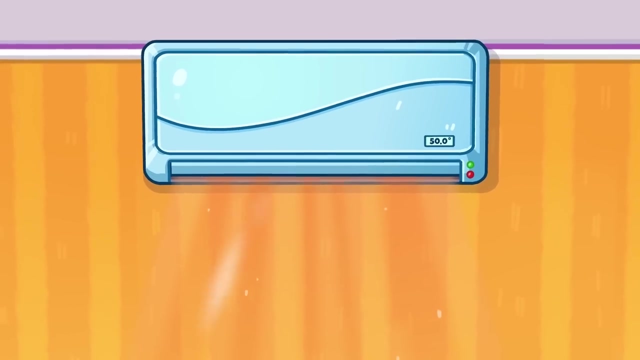 Ah, Ah, Ah, Ah, Ah Ah Ah. The sun is too hot today. It's even too hot to play outside. Everyone should go inside the house. It is dangerous to play outdoors when the temperature is high. Inside, you can use a fan or air conditioning to keep cool. 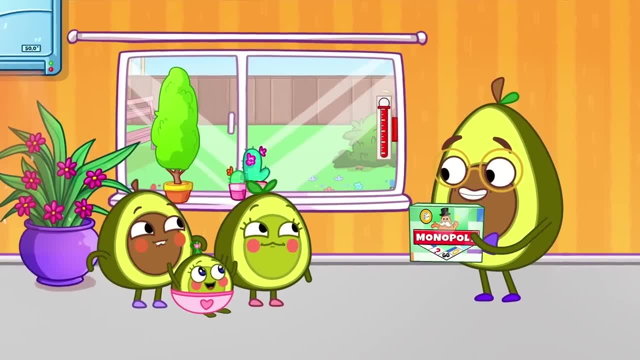 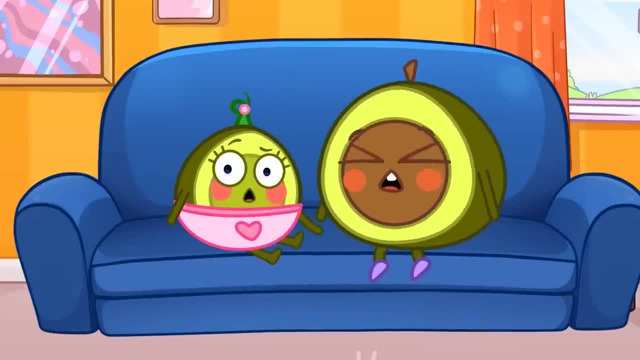 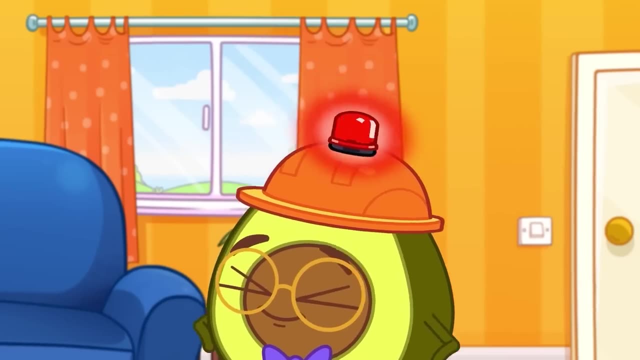 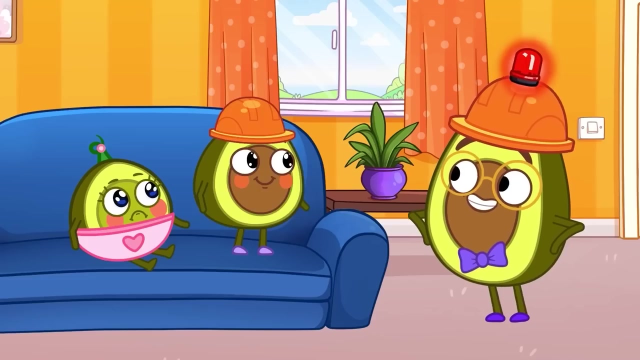 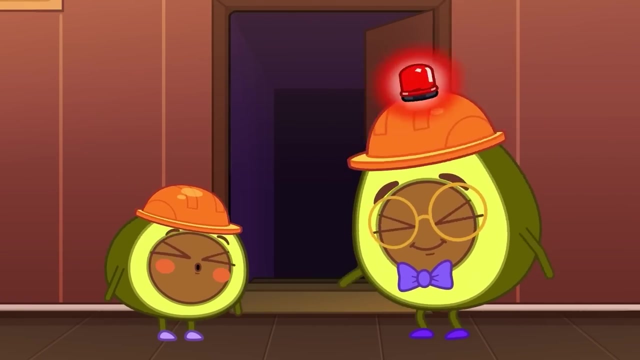 You can play at home. What a great idea, Daddy. Oh no, What happened to the TV? Who will fix the TV? Don't worry, Dad will help And I'll be your little helper First. First you have to go into the basement. 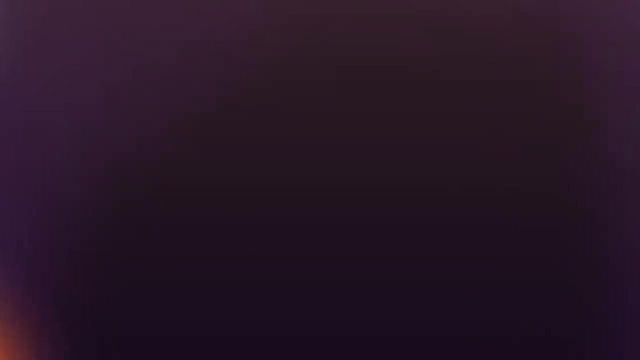 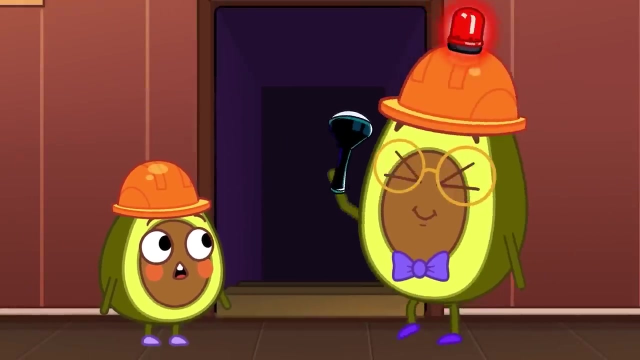 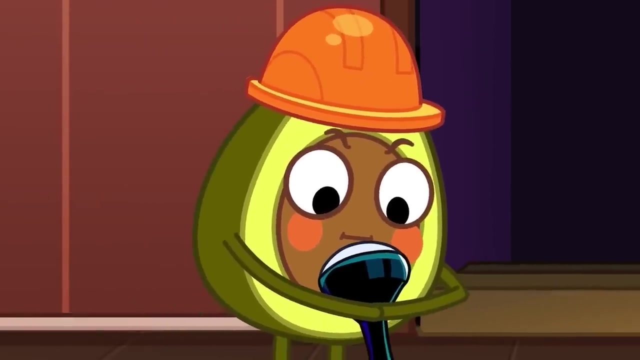 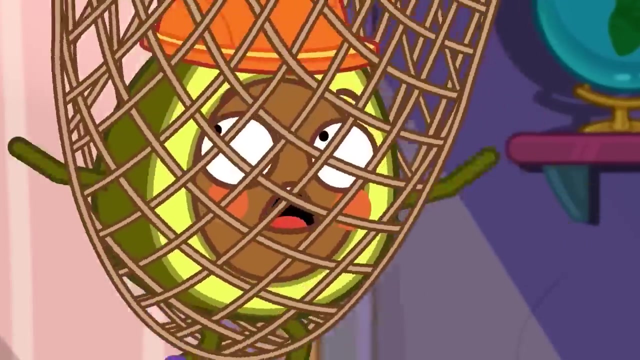 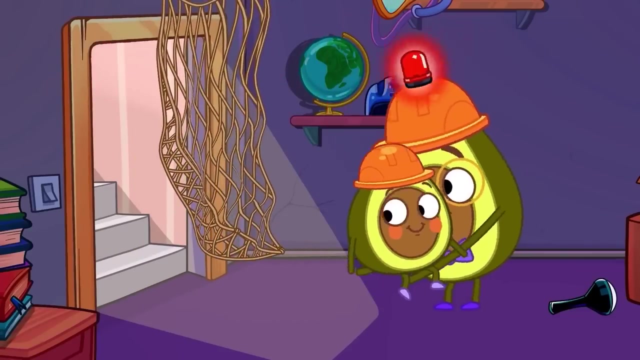 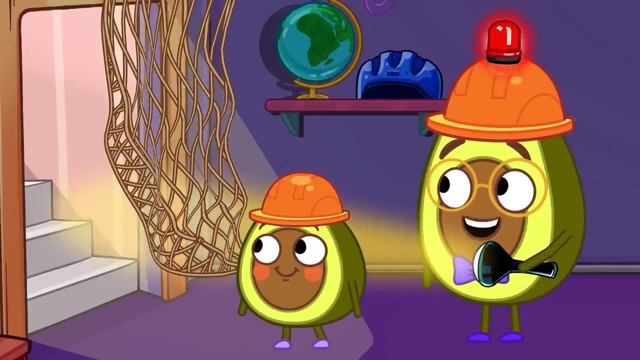 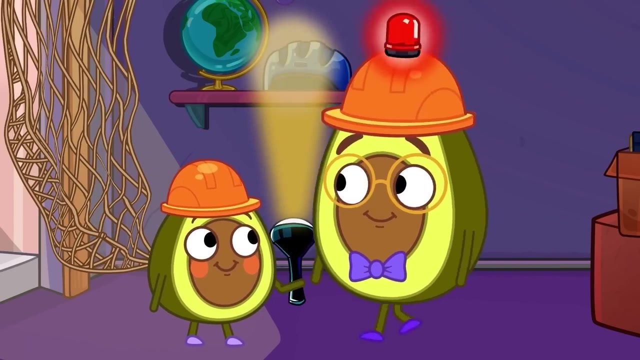 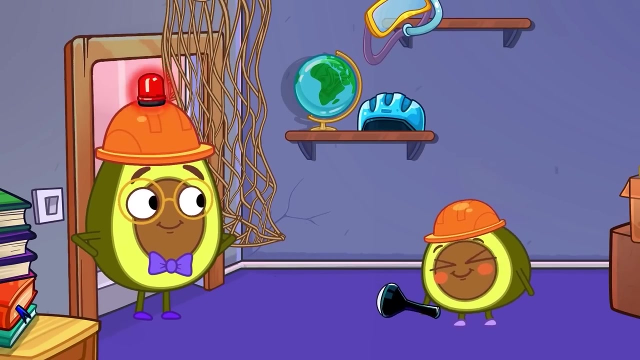 But it's dark and scary down there. Maybe a flashlight will help. It's caught, Monster, help me. You're safe now, Pit, There are no monsters here. Look, It was just a net. Daddy will check the electrical box. 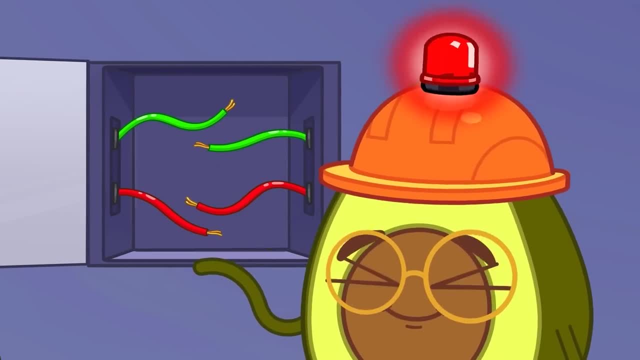 It's a very powerful one. It's like a mini-newscast. Wait, I can't, It's a full house. There's nothing. Where's the TV? I'll come check it out And maybe I'll help you fish. 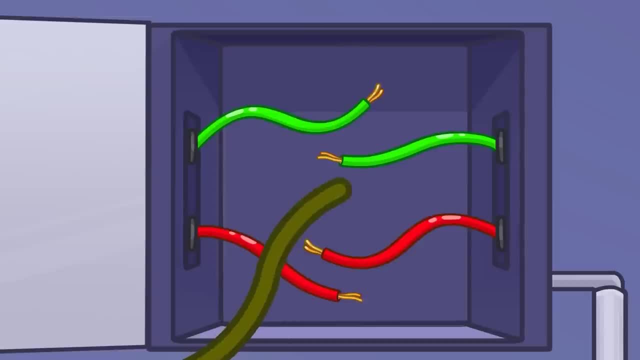 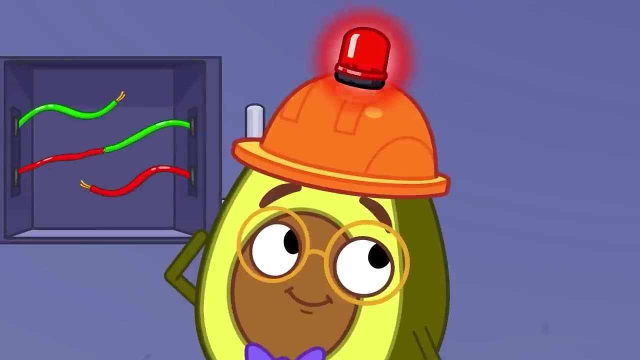 I'll make a wish for you. What, What are we going to do? Maybe we can use that little bell. The wires are loose, OK, Ooh, They need to be reconnected. The TV still doesn't work. Should we connect them in some other way? 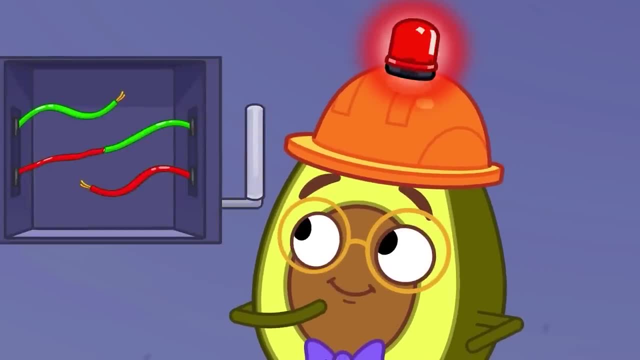 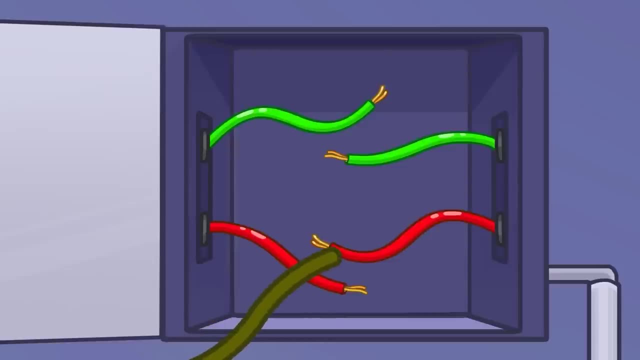 Ready, Here we go. Who goes to dinner first Me, or you Me, Me first, Me first? Who goes to dinner first Me first? Me first, Me first? Who goes to dinner first Me first? Red goes with red and green goes with green. 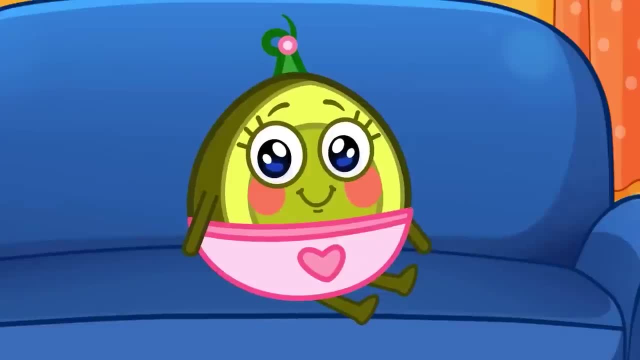 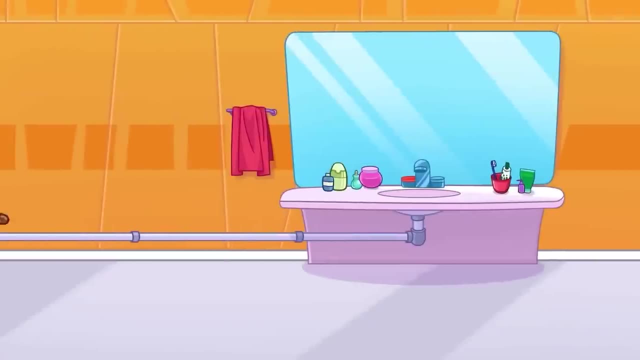 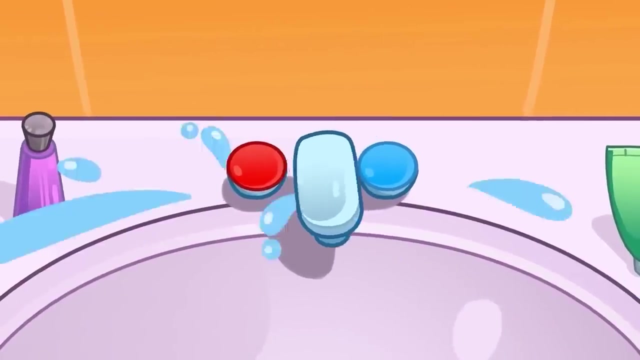 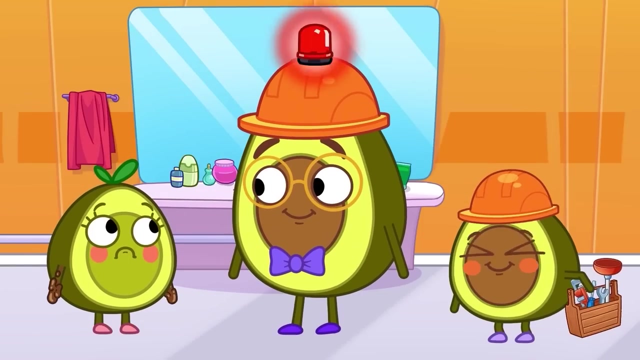 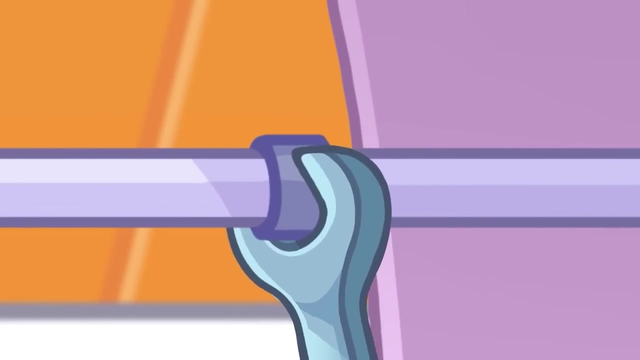 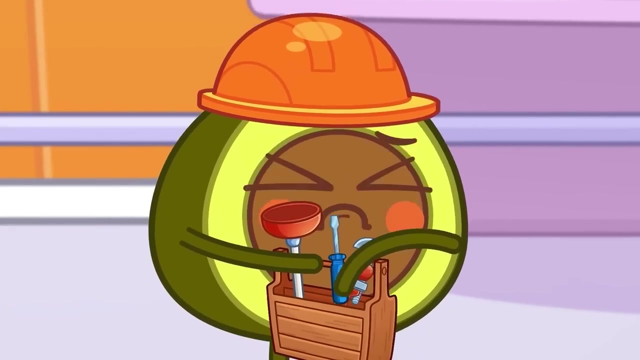 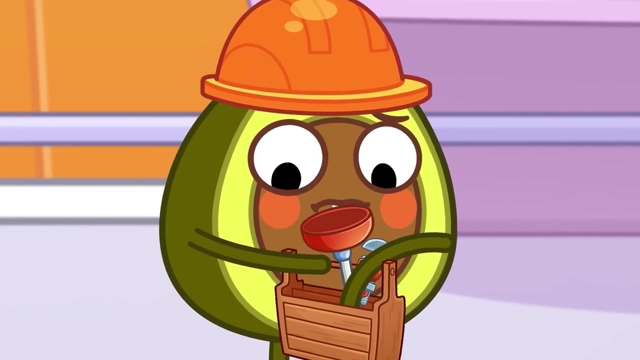 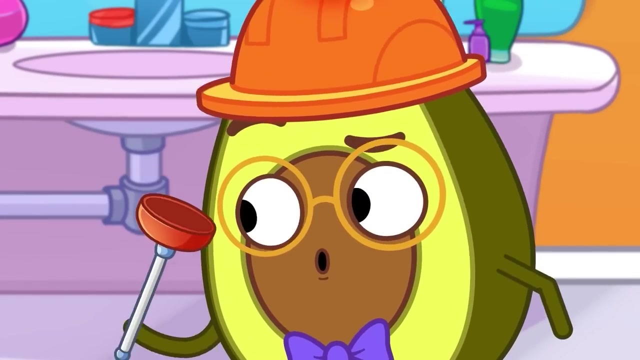 It worked. Penny wants to wash her hands. Oh oh no. How can I wash my hands now? We'll fix it, Babe. I need another wrench. That's a screwdriver And that's a plunger. It's stuck on Daddy's head. 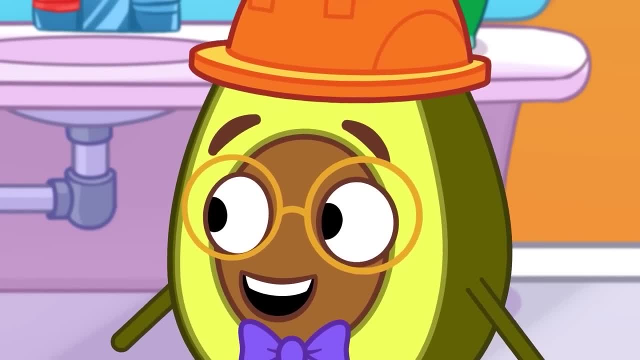 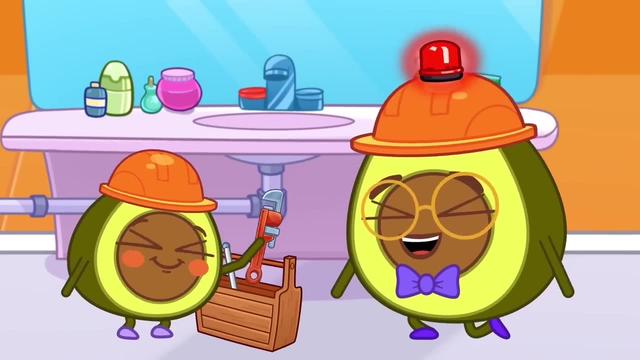 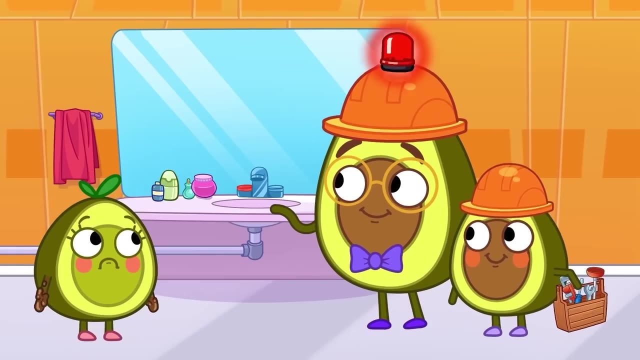 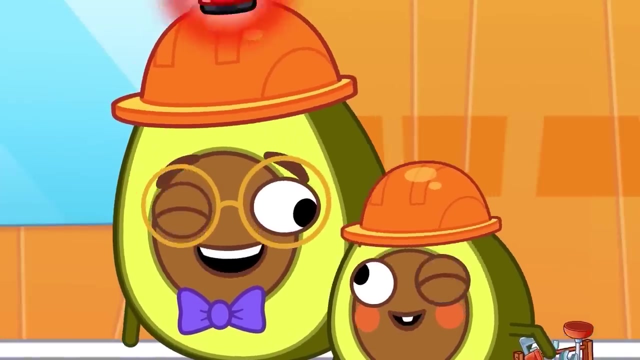 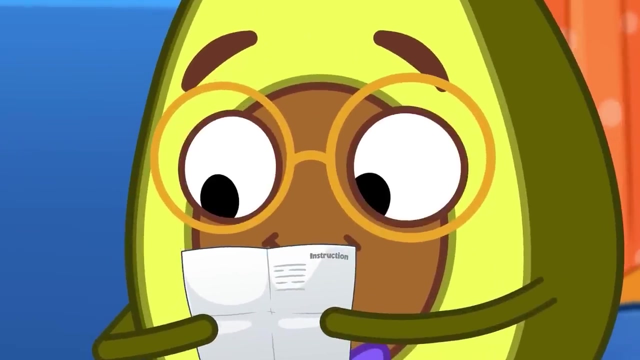 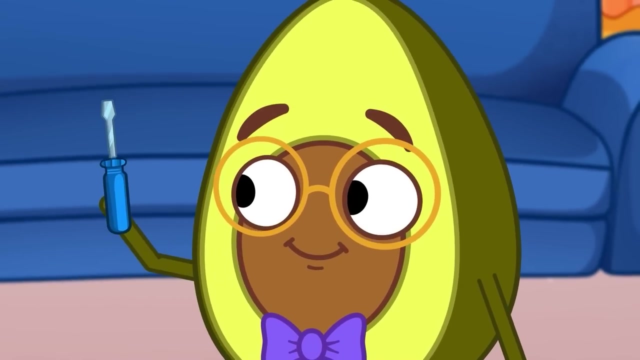 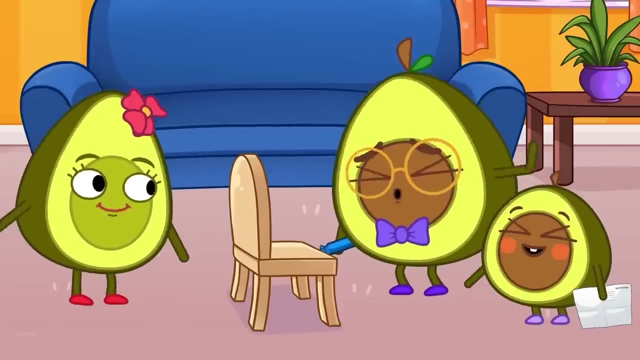 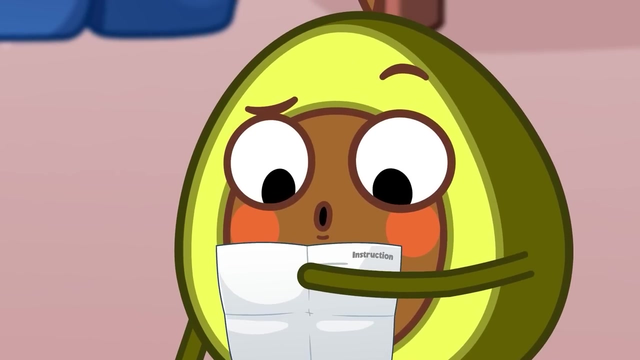 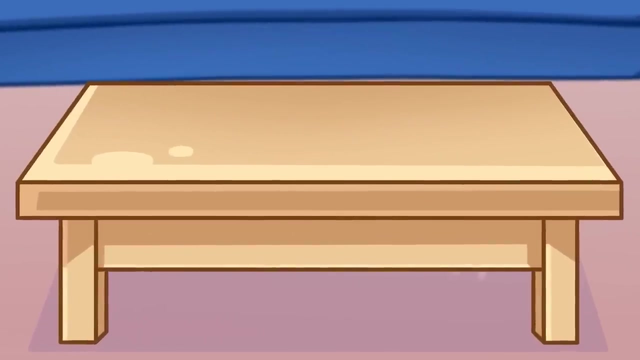 Phew, That's better. Yes, that's the wrench Daddy needs. The sink is fixed. Mommy needs help building a cabinet. A cabinet, Daddy can do it. That's not right. Maybe, Oops, Wrong again. Maybe you need another tool. 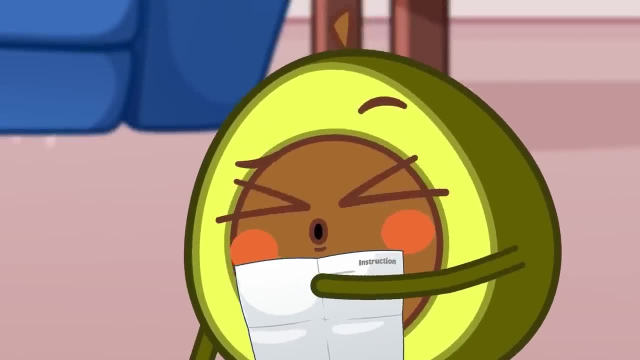 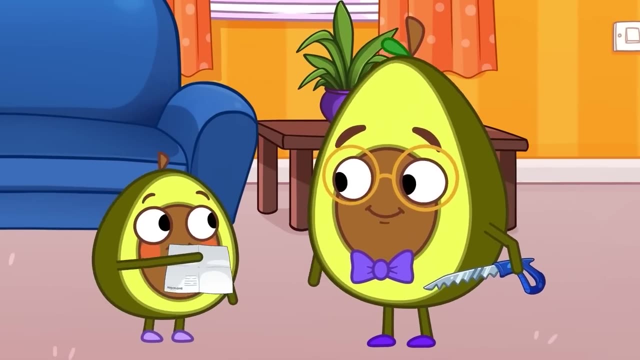 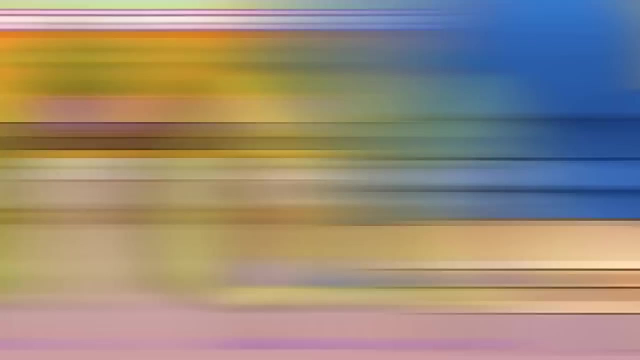 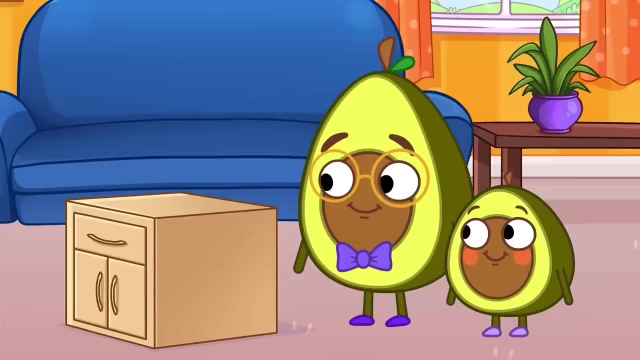 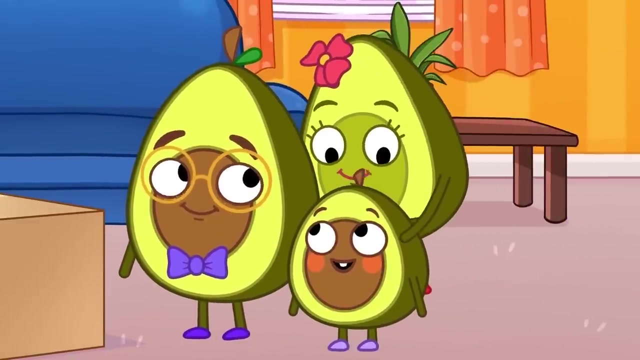 Huh, Huh, Huh, Hmm. Oh, Pit knows what's wrong. Hmm, Uh-oh, This is how it's supposed to work. The instructions were upside down. That's much better. Ah, You're a daddy's little helper. 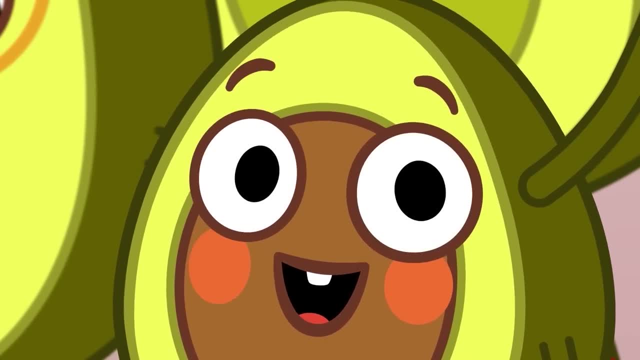 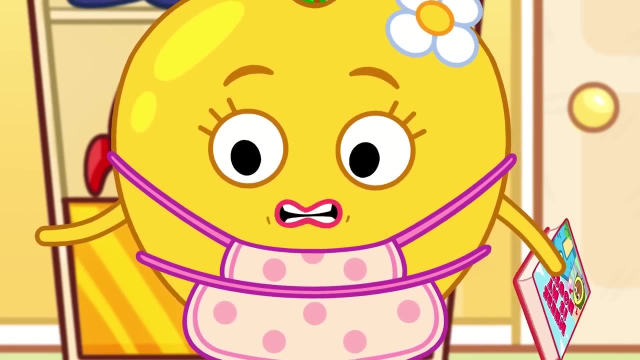 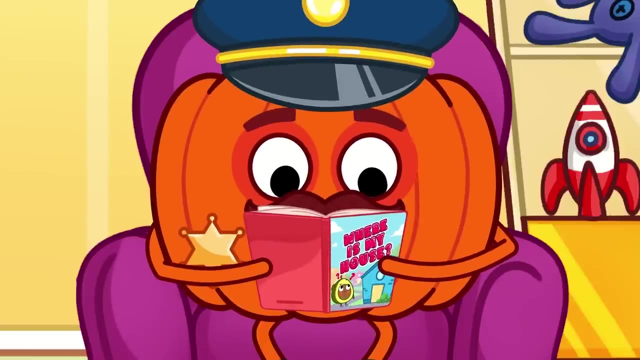 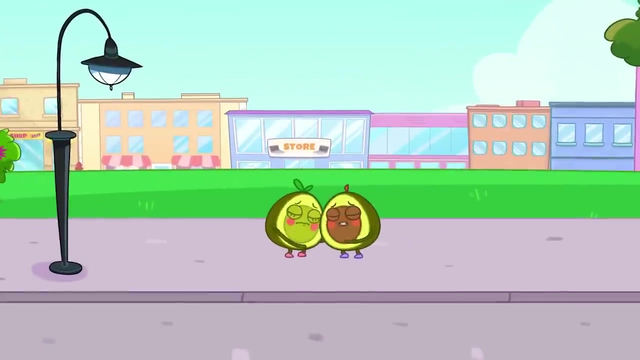 Well done Pit Phew Children. today, the officer will read you a fairy tale. The children like fairy tales. Once upon a time, Pete and Penny forgot where they lived. Oh no, Hey, hey, hey, Oh no. 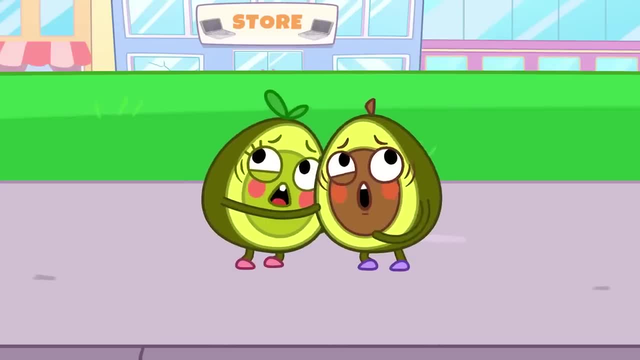 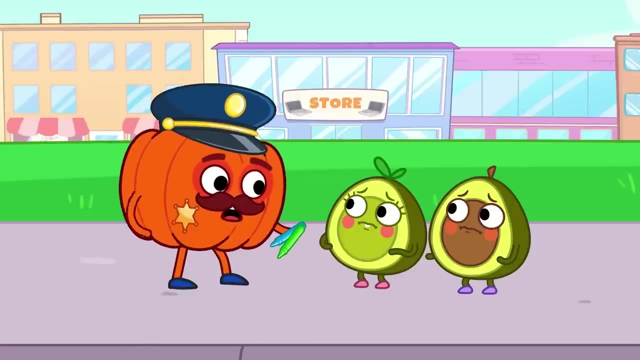 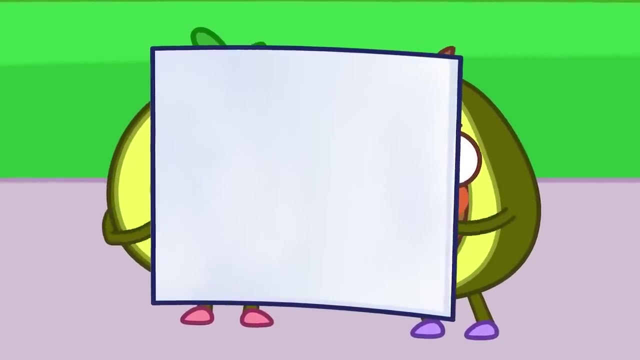 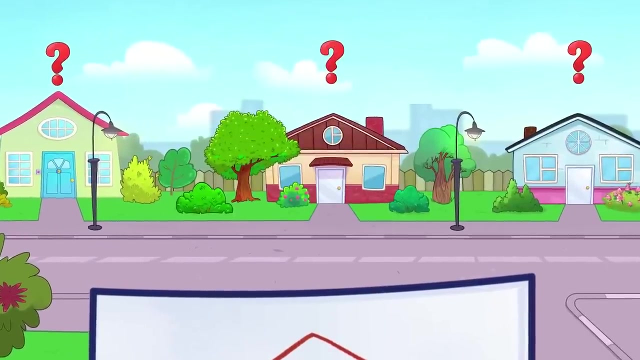 Pit and Penny are lost. Help us Help. Huh, Are you lost? Children, Can you please draw your house for me? Officer Pumpkin is trying to help. That's a very pretty drawing. Officer Pumpkin is looking for Pit and Penny's house. 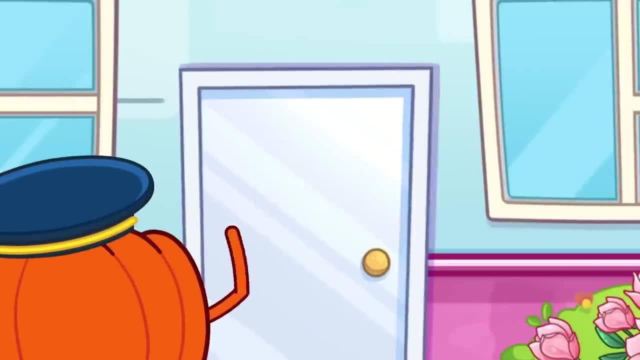 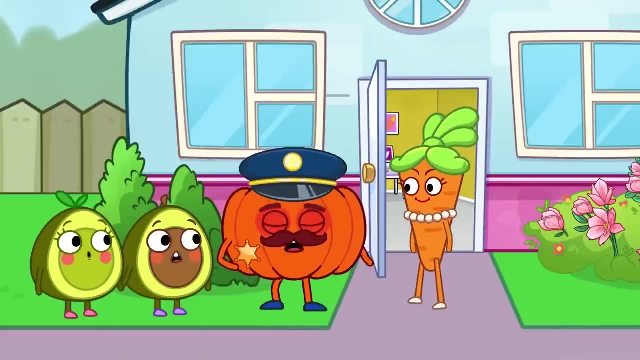 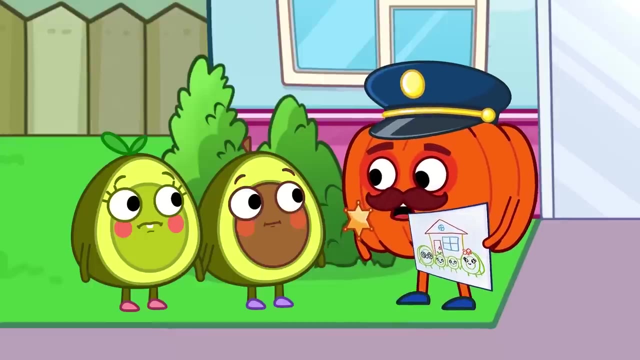 Ok, Let's try to find your house. Oh, You're such a good boy. Is this Pit and Penny's house? Are these your parents? That's Mrs Carrot. Does your house really look like this? Let's try over there. 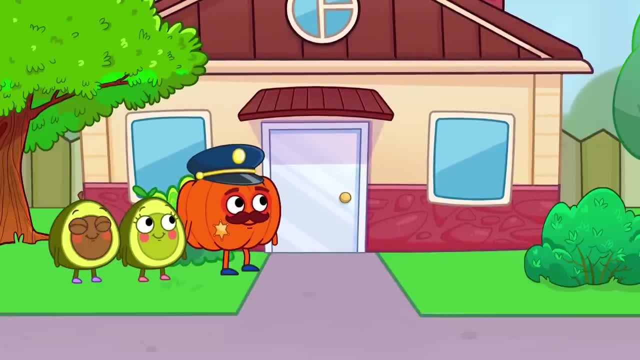 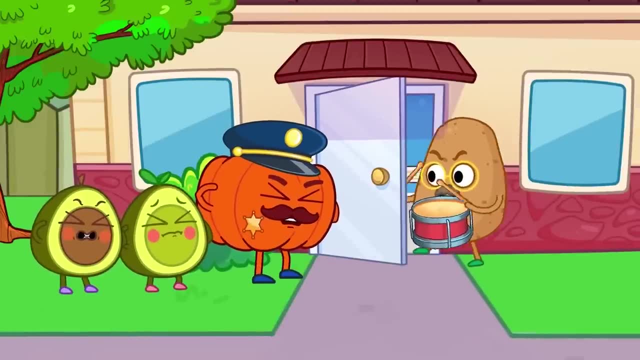 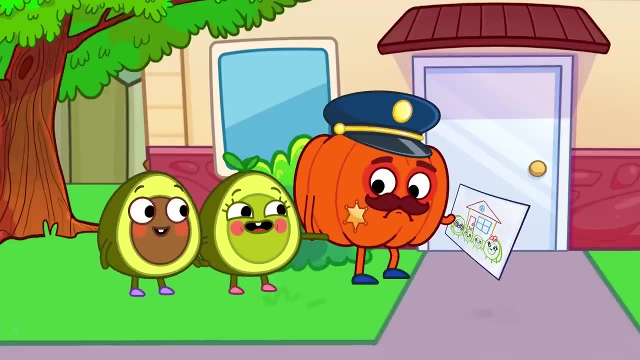 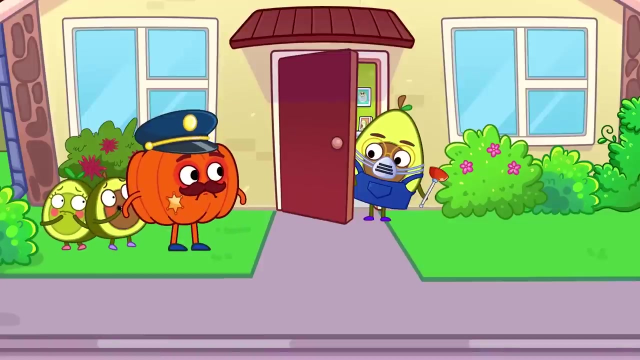 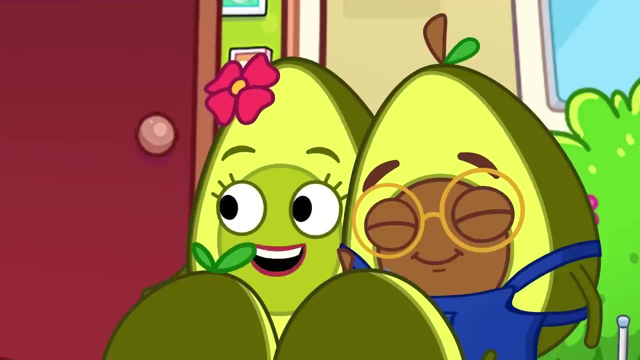 Maybe this is Pit and Penny's house. Are these your children? The drums are very loud. What have you seen, Penny? Pit and Penny are scared. It's Mommy and Daddy Officer. thank you for bringing our children back home. 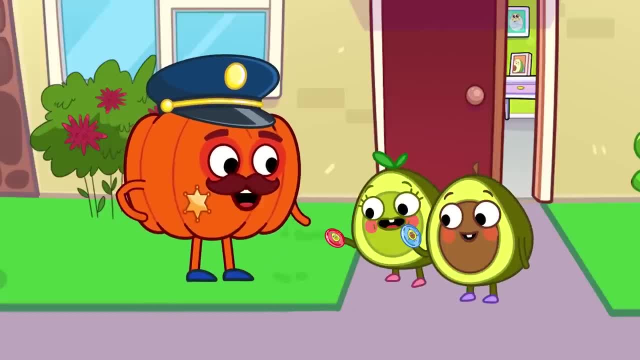 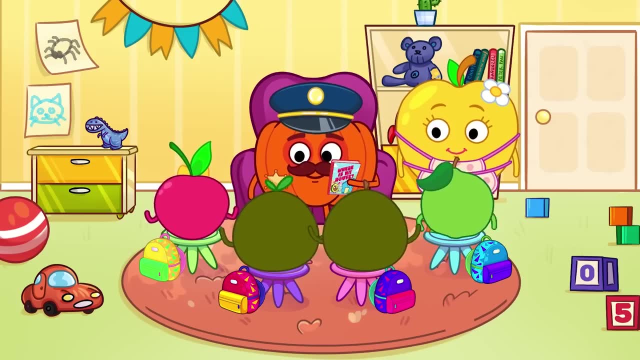 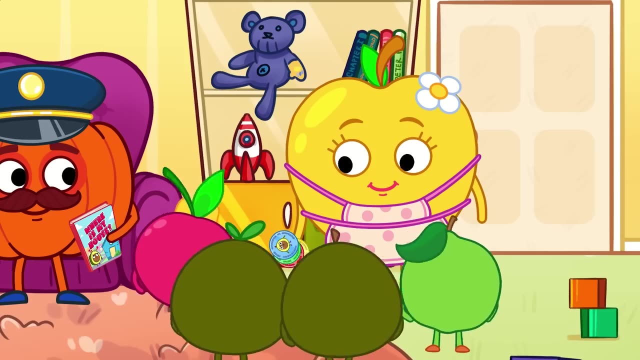 Officer Pumpkin has a special gift for Pit and Penny. Your address is written on the badges I gave you. What a story. Kids keep your badges with you so you can always find your way home if you get lost. It's a happy ending. 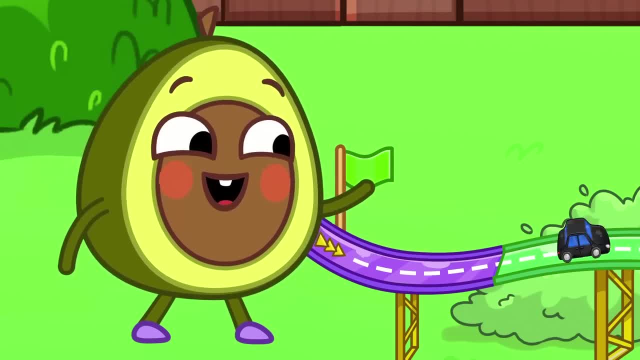 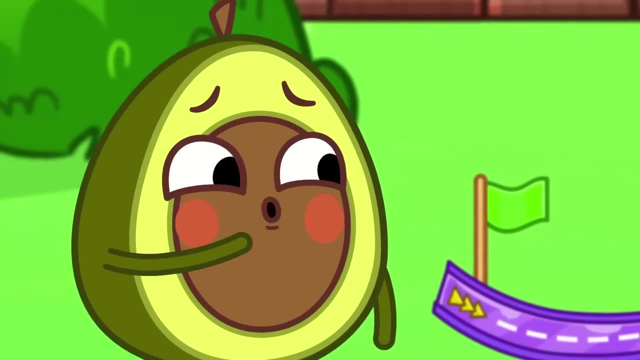 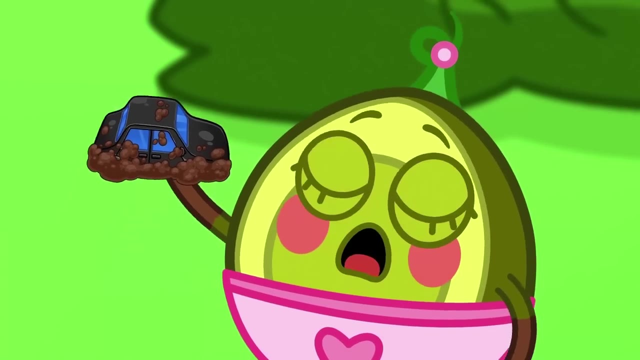 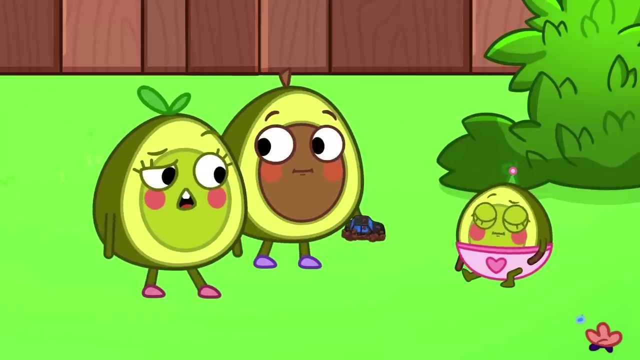 Pit and Penny are playing with their toy car. It landed in a mud puddle. Oh no, What's Baby going to do? Stop, Don't put it in your mouth, It's covered in yucky germs. You must wash your hands. 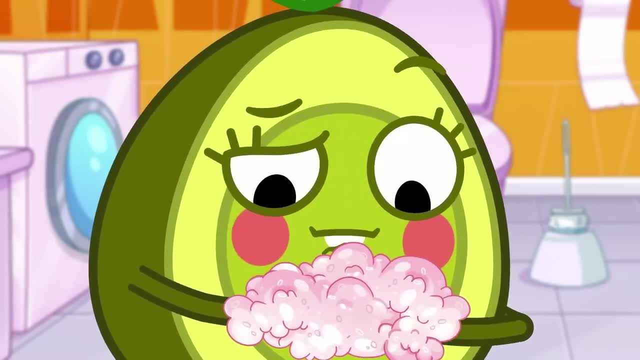 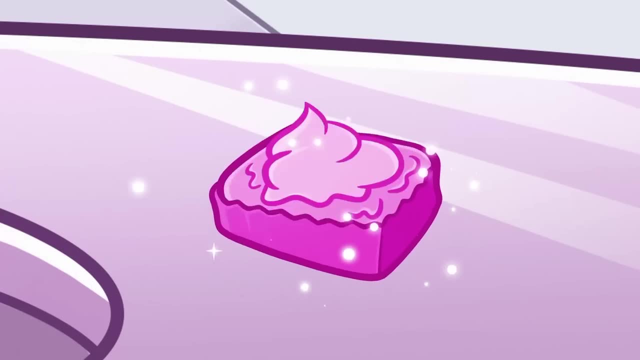 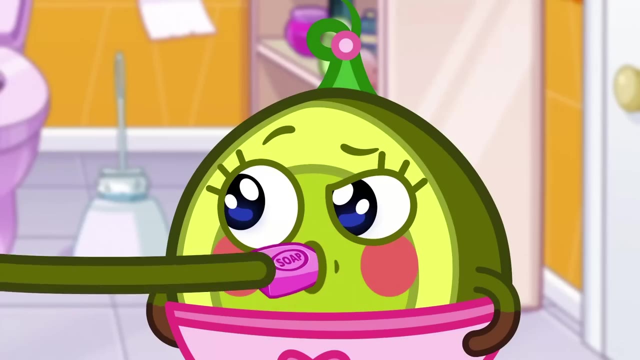 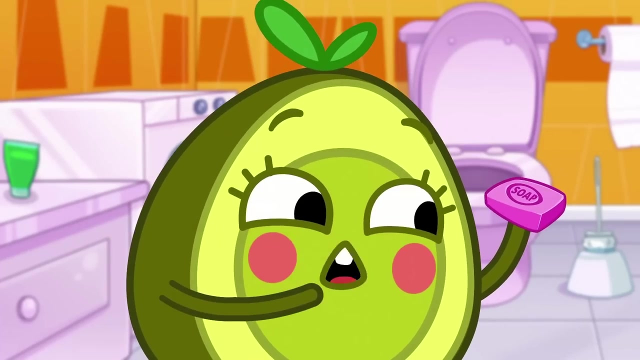 First let's wash the car. Baby thinks the soap looks like cake. Oh no, Stop, Don't put it in your mouth. Tell her why. Penny, The soap looks delicious but it's not edible. See, No more germs. 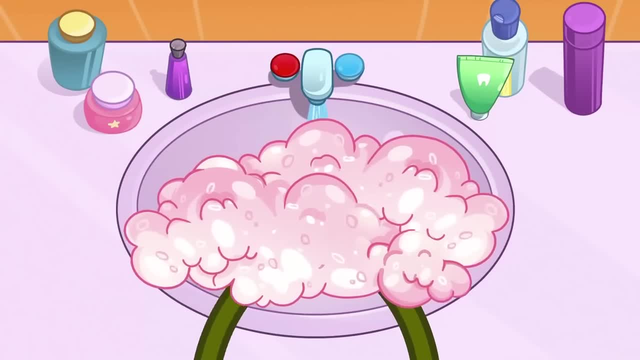 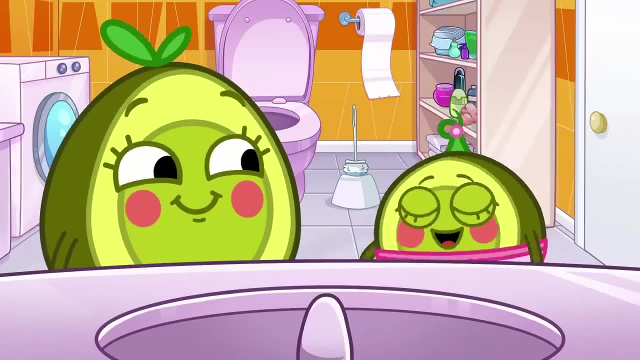 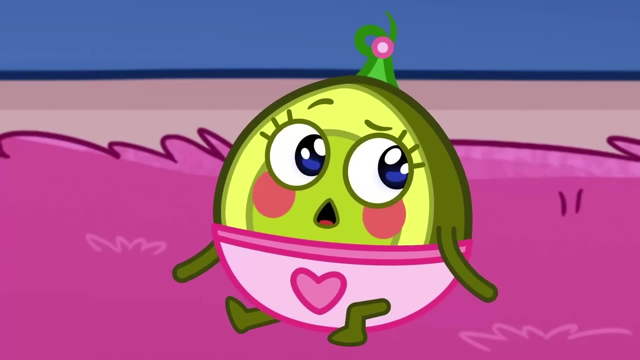 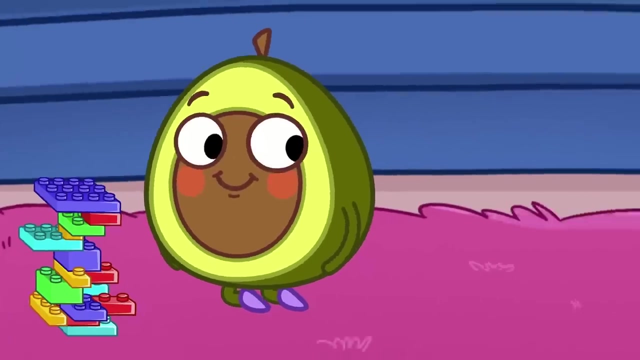 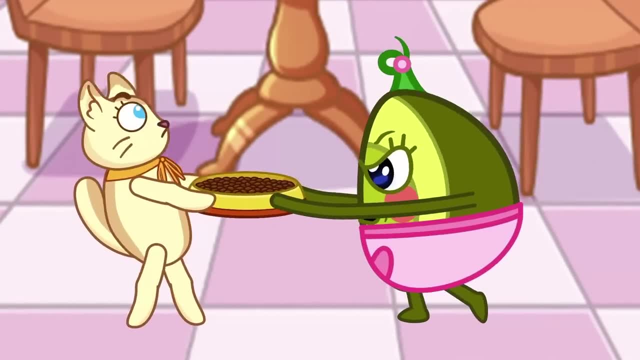 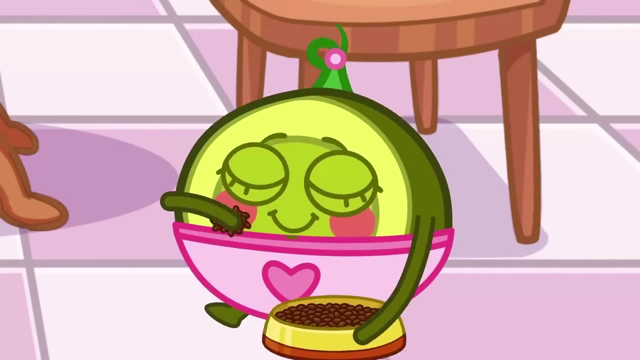 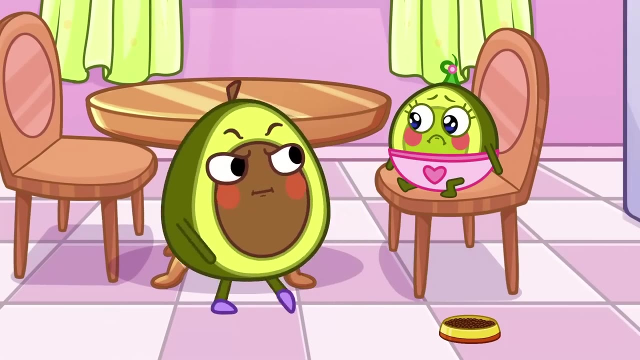 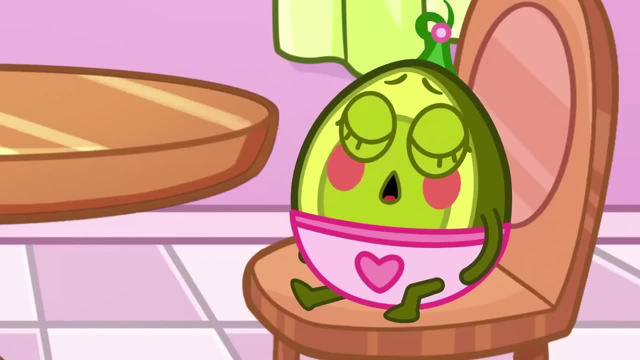 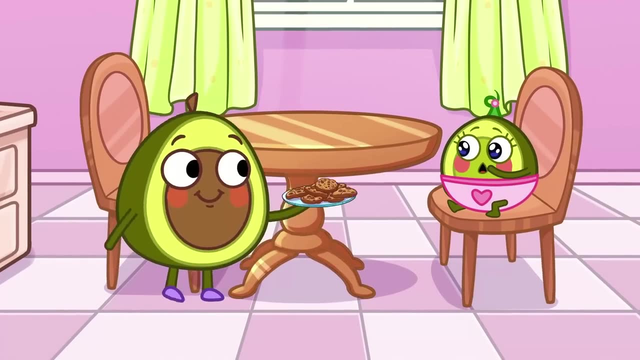 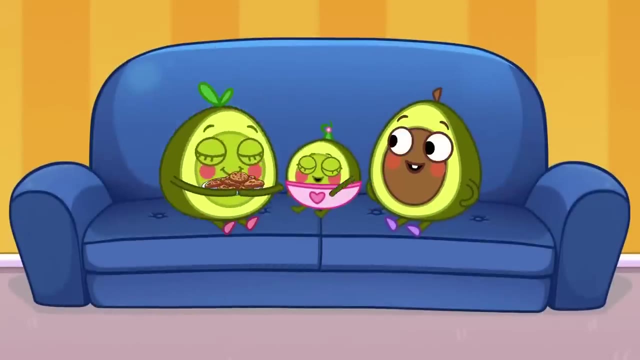 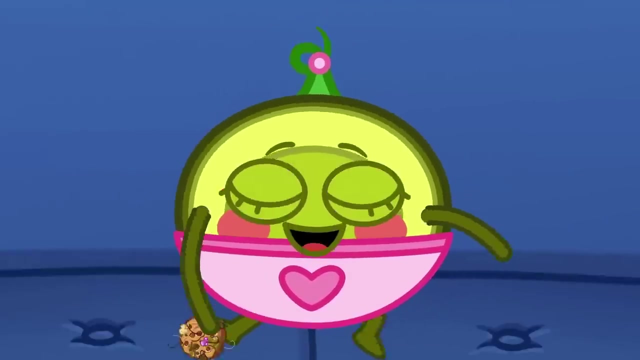 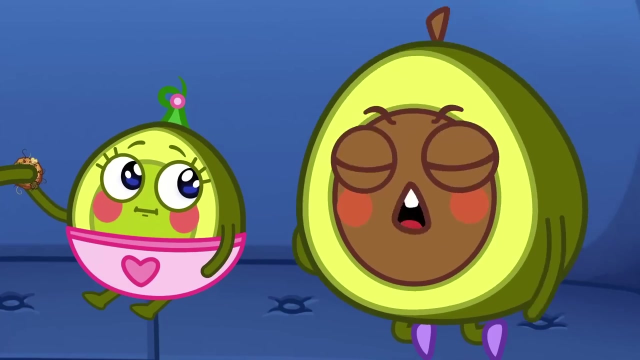 This food is only for pets. We can't eat it. Look, Pit has cookies. Look, Pit has cookies. But we can eat this. But we can eat this, But we can eat this. That cookie looks dirty. Stop, Don't put it in your mouth. 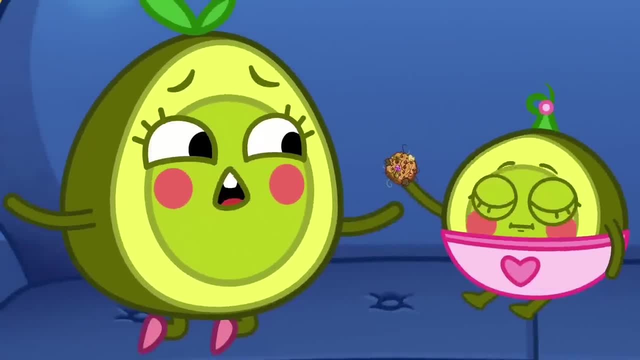 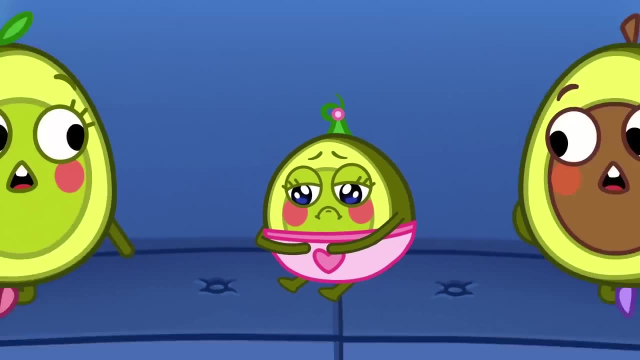 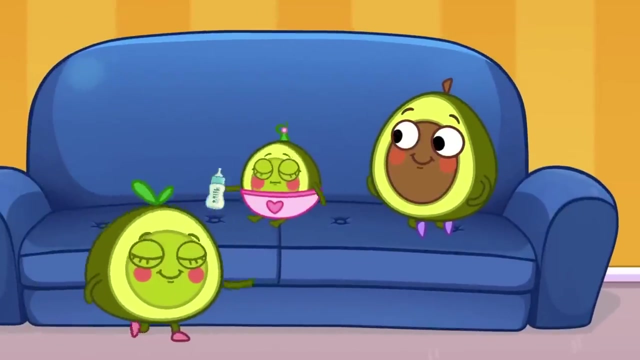 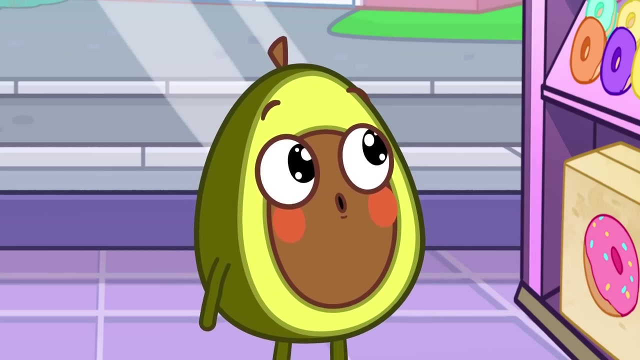 You can't eat food that fell on the floor or sofa. It might make you feel sick. Baby is very hungry. Penny knows what to do. A bottle of milk will make Baby happy. Pit and Penny are helping Mommy shop And Pit thinks they should get junk food. 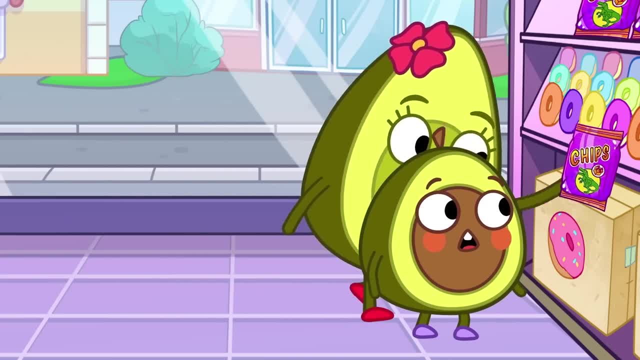 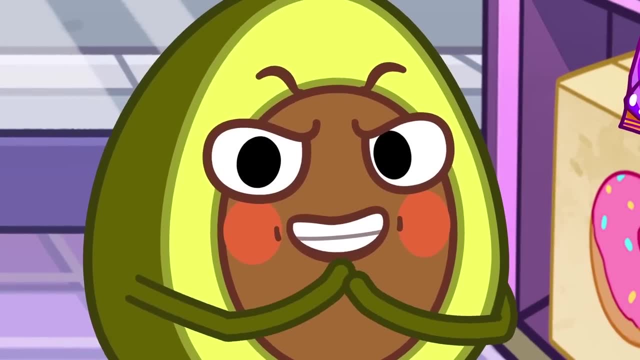 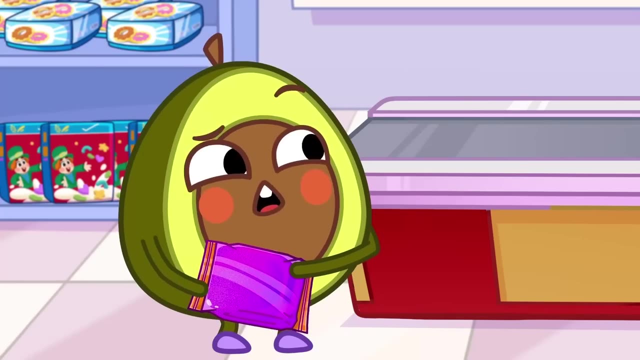 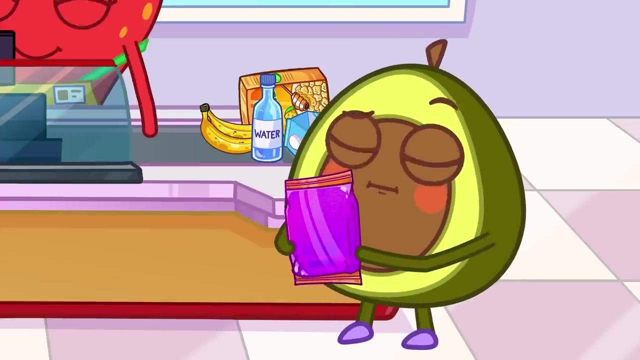 These snacks are unhealthy. Sorry, Pit, Junk food is not good for you. Pit has a plan. While Mommy is paying for groceries, Pit sneaks his junk food onto the counter. Oh Pit, It's bedtime. Good night, kids. 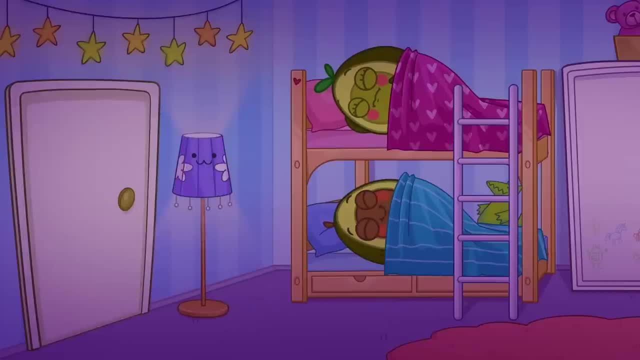 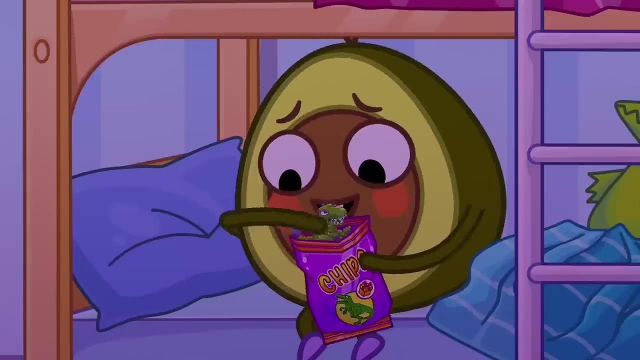 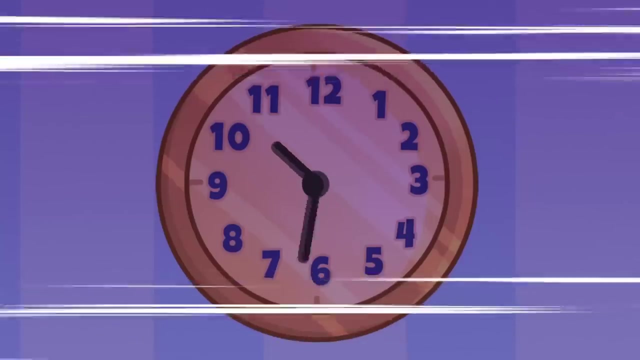 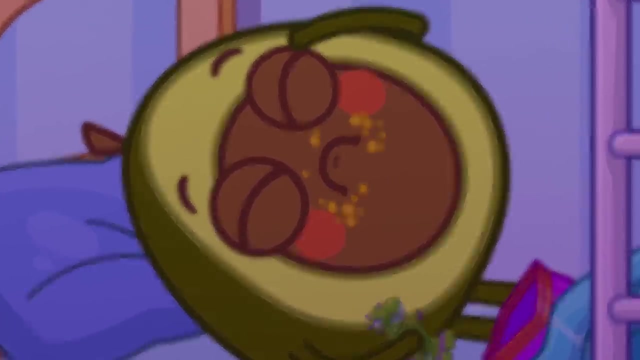 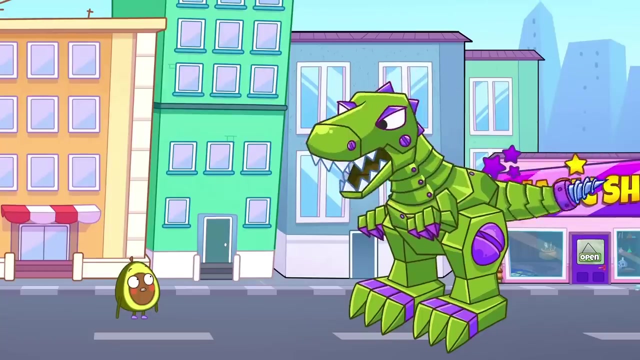 Good night, Mommy, But Pit is not ready to go to sleep. He wants to eat his chips. Be careful, Pit, or you'll get an upset tummy. Pit is having a dream. Yikes, It's the T-Rex 2000!. 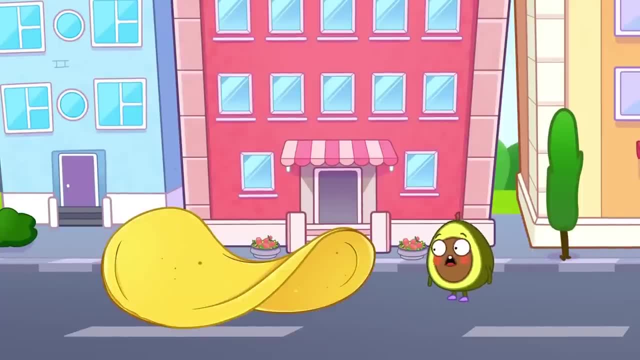 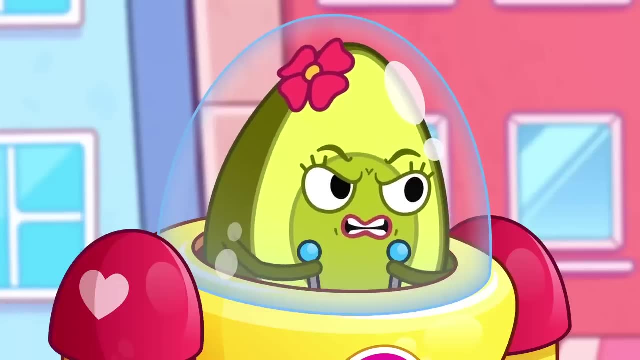 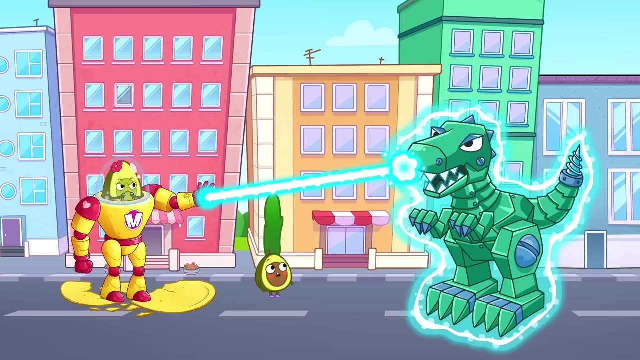 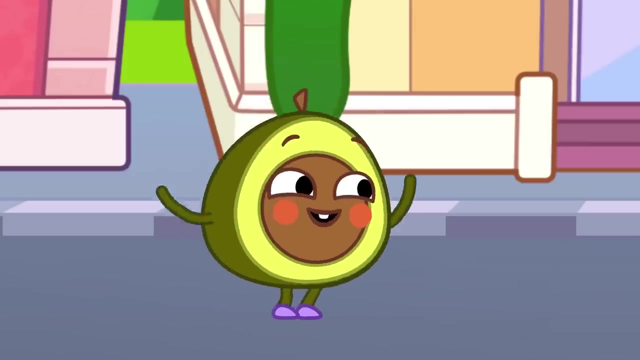 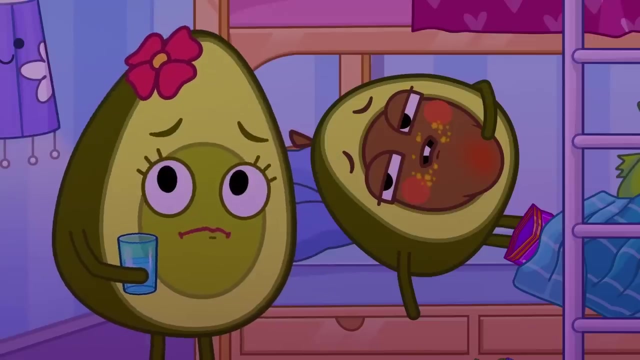 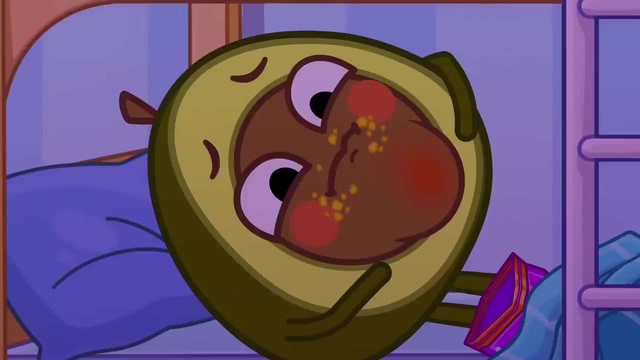 Run Pit. Who will save Pit? now Let's go Pit Super Mommy to the rescue. Watch out, Mommy, Everyone is safe. Pit has a tummy ache. Mommy will save the day Again. Thank you, Mommy. 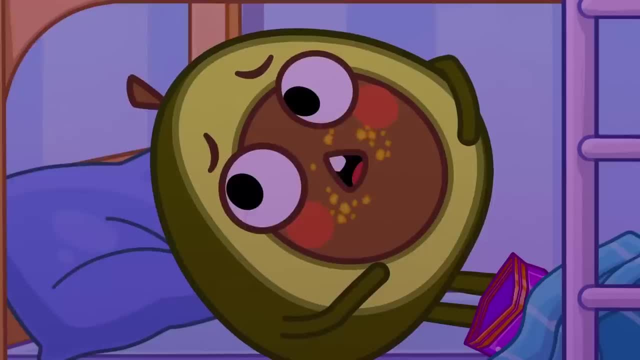 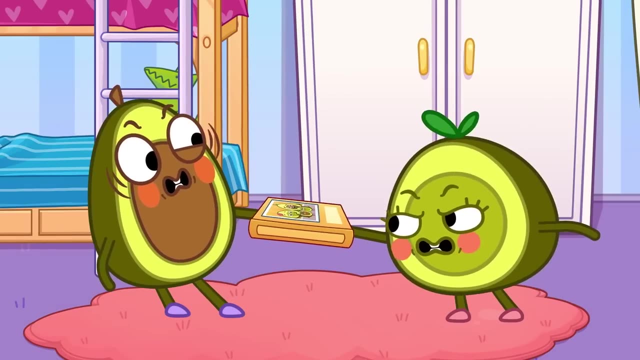 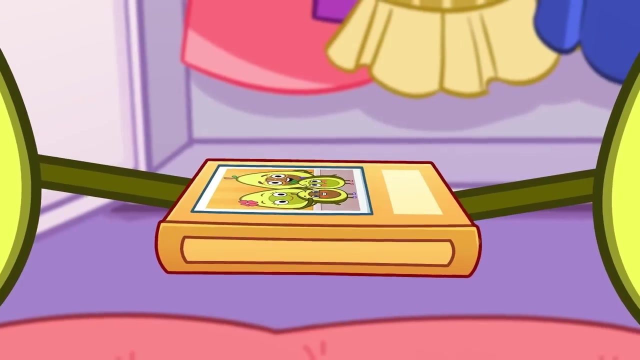 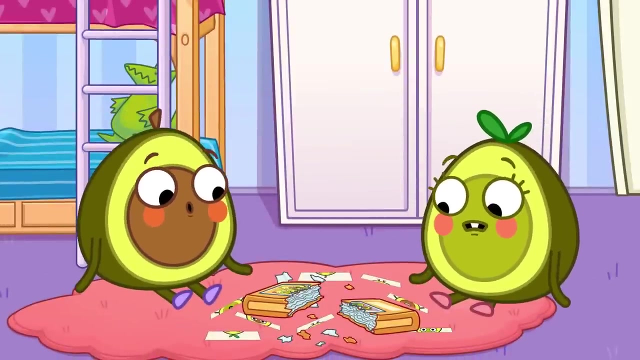 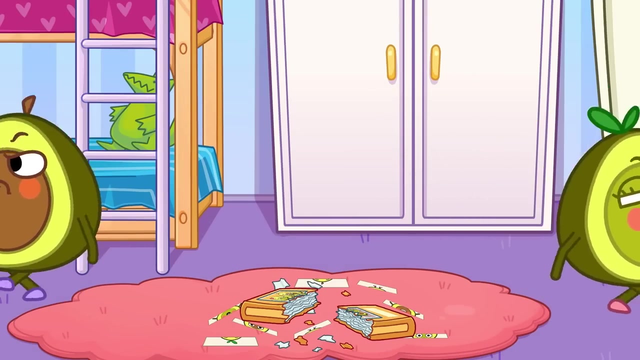 Pit, don't eat unhealthy snacks. Okay, Night-night. you two Stop fighting kids. These photos are mine, No mine. The photo album is ruined. Pit blames Penny And Penny blames Pit. Here comes Baby. She loves looking at photos. 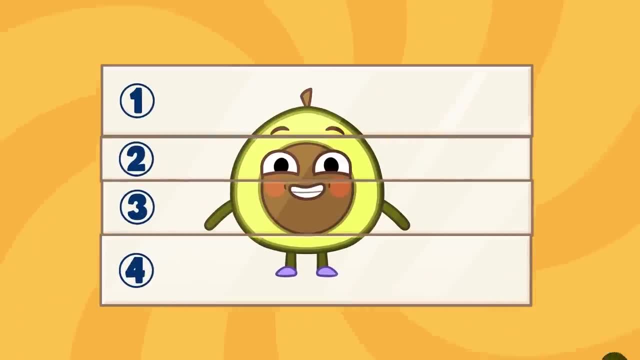 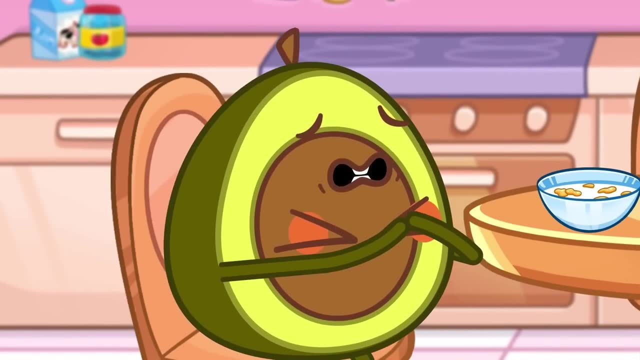 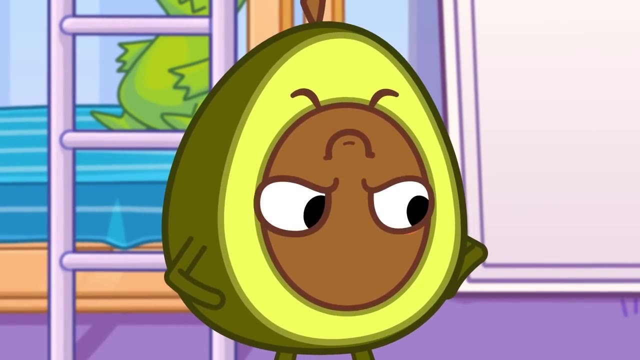 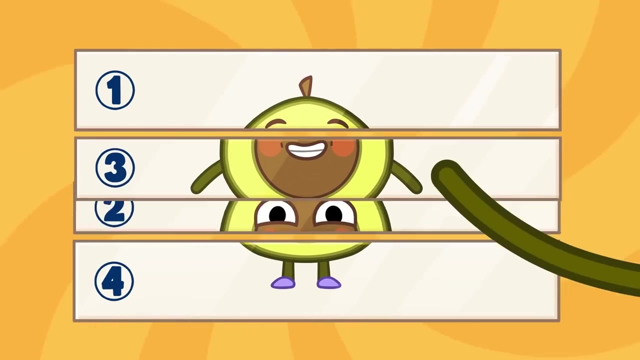 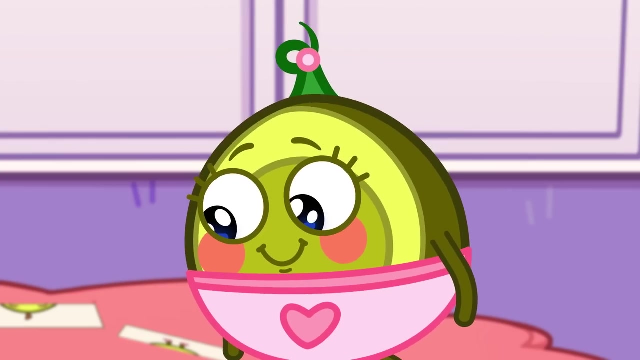 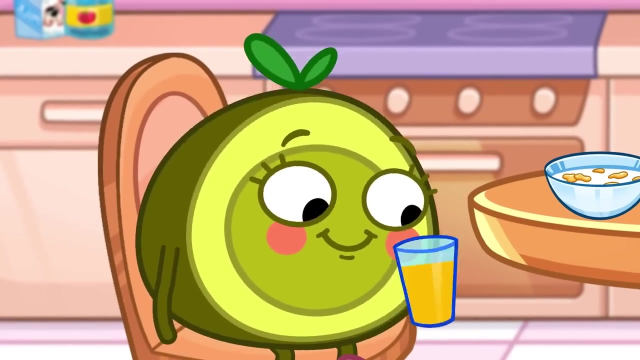 Can she put the pieces in order? Whoops, that's not right. Let's fix Pit's face. Baby, Can she do it? Of course she can. This is a picture of Penny Now. Penny has a kitty face, Oh. 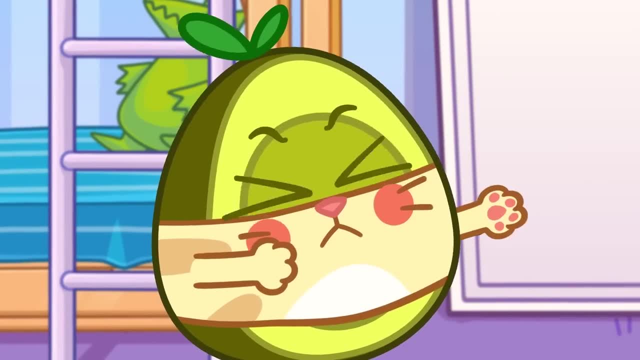 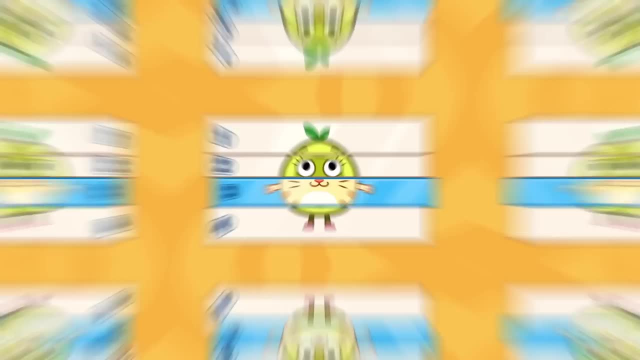 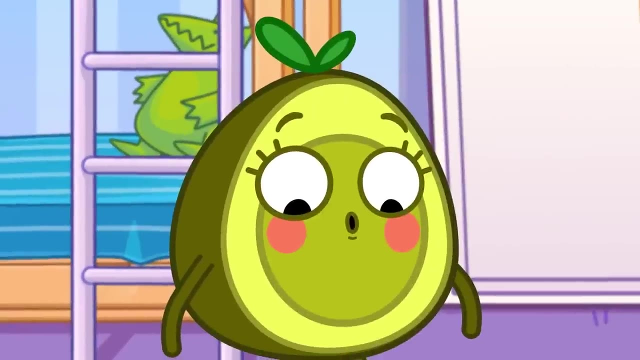 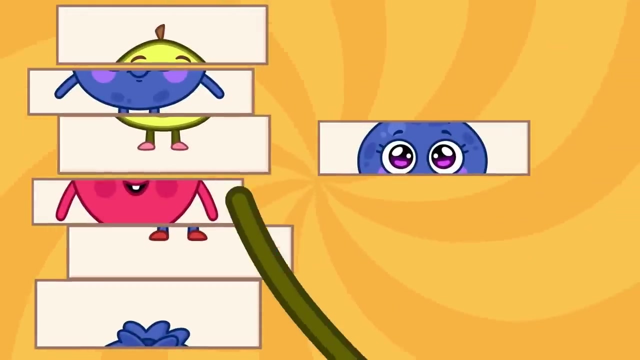 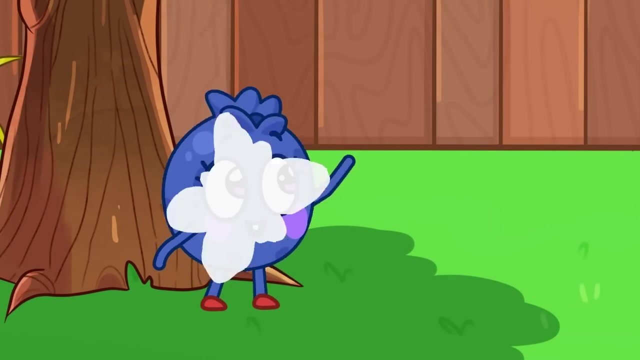 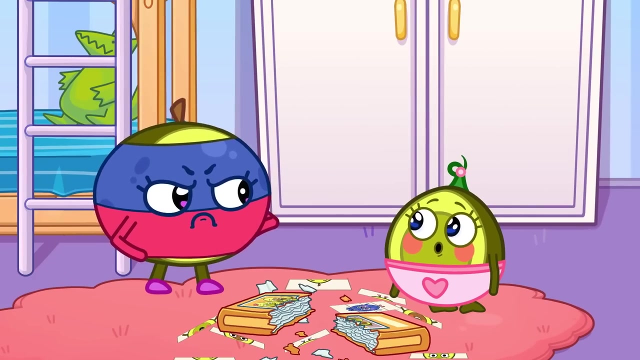 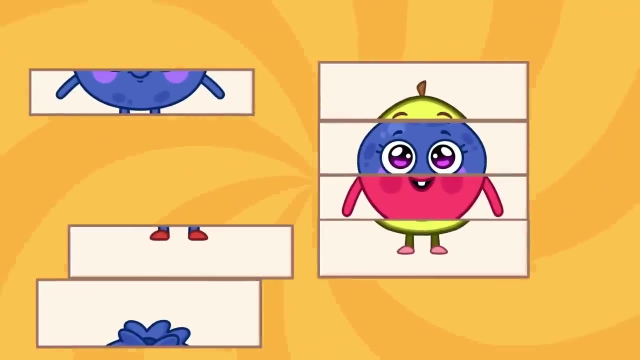 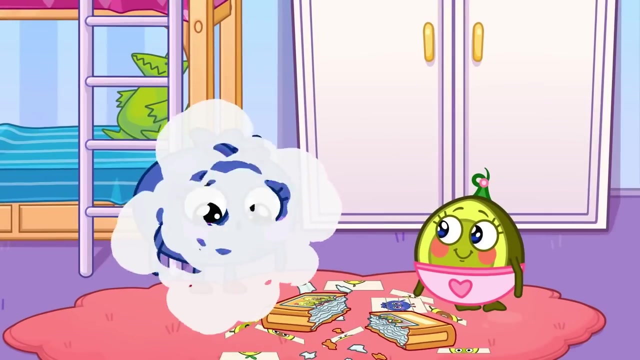 Can Baby fix Penny's face? Of course she can See. That's much better. What is she doing to Blueberry? That's not right. Blueberry isn't very happy. Don't worry, Baby knows what to do. Yay, Blueberry is back to normal. 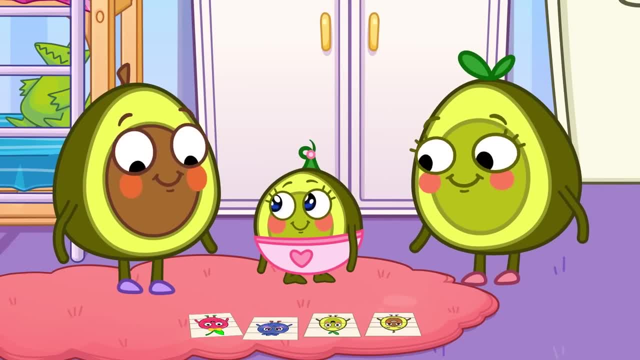 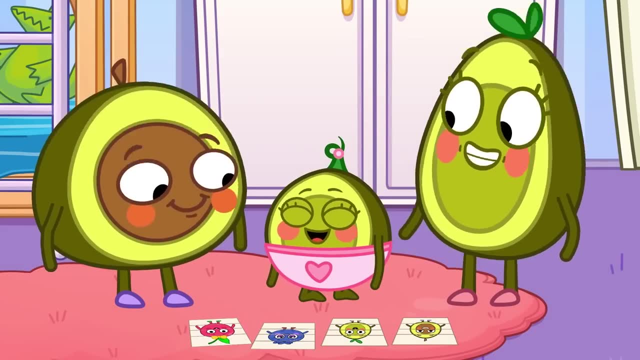 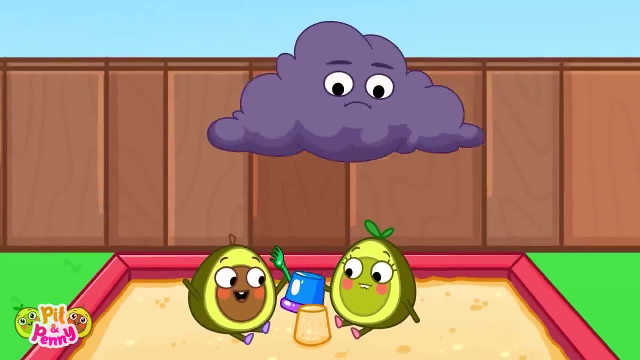 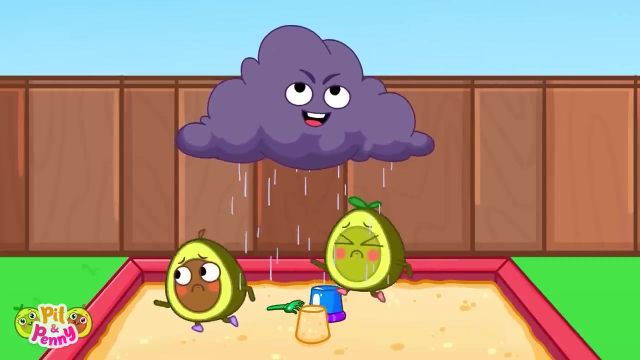 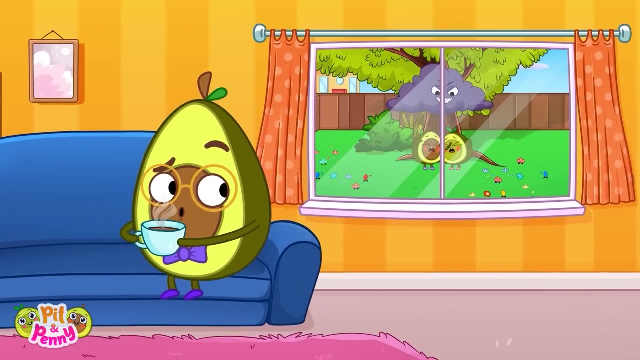 Look what Baby did kids. She has put the photos back together. Good job, Baby. The kids are playing in the sand. A rain cloud- What a mean cloud. Daddy is trying to relax. Look, Daddy. Pit and Penny need you. 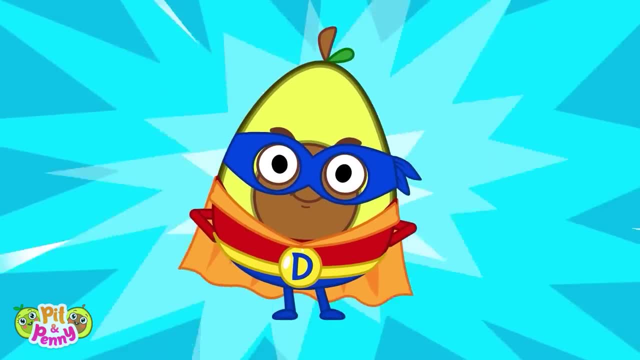 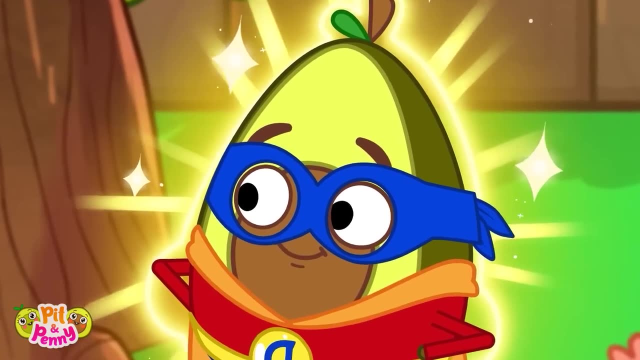 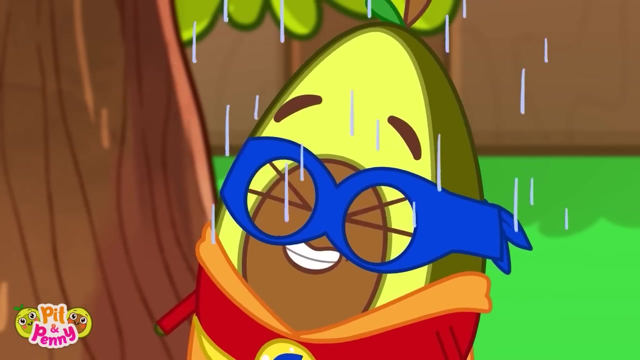 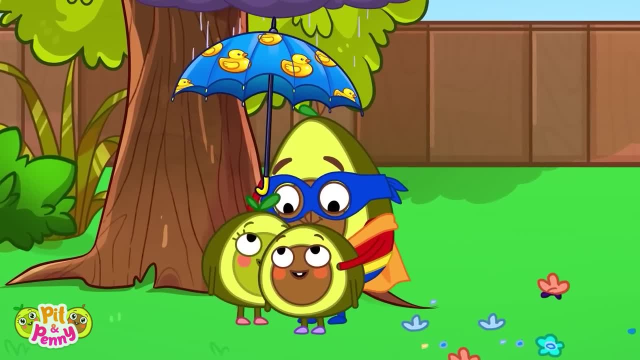 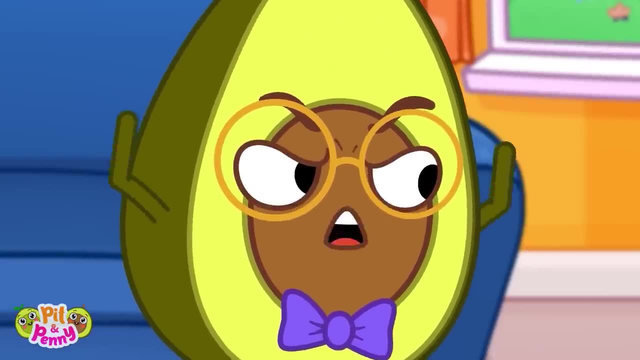 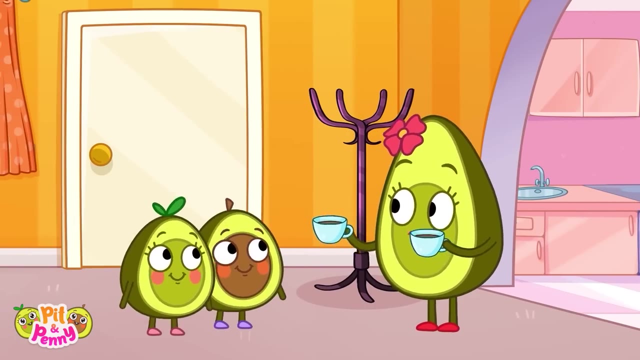 Oh no, The umbrella blocks the rain. Bye-bye cloud. Kids do not stand under trees in bad weather. It's dangerous. I'm sure Pit and Penny won't forget. Now Daddy can relax. What character reminding us to push forward. 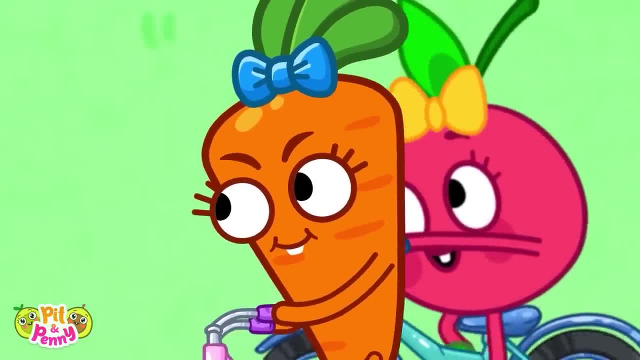 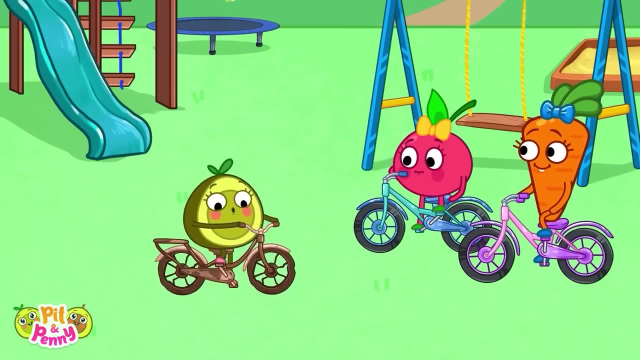 Cherry and Carrot are racing their bikes. I hope to go in all its glory…. Penny's bike is old and rusty… And broken… A reflect can make us go anywhere. it's like a motorcycle For Penny. Daddy is gonna protect her…. 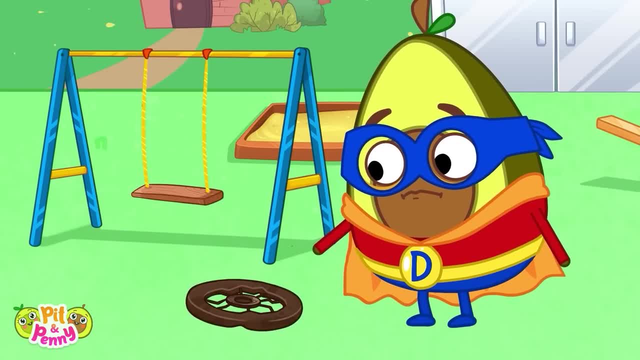 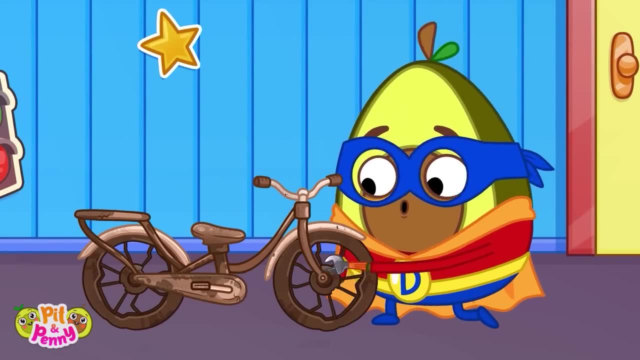 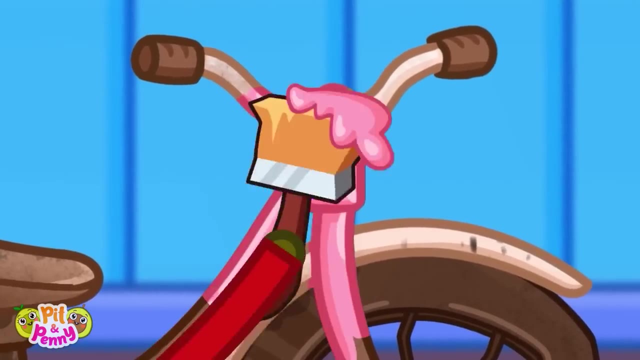 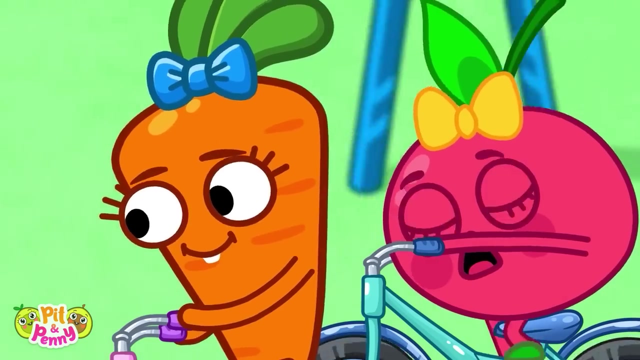 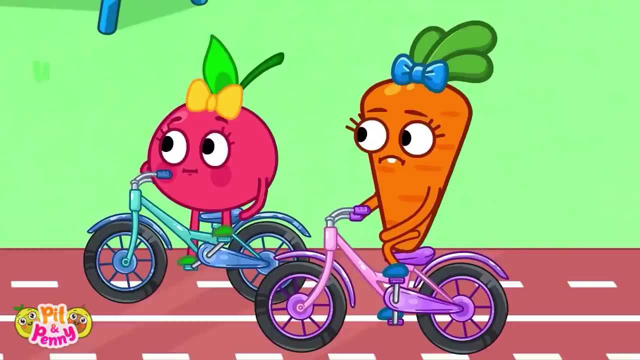 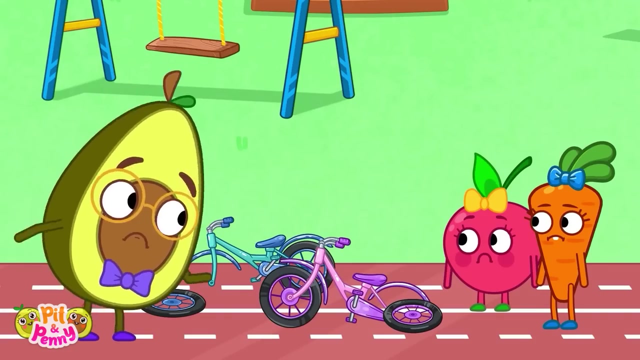 Poor Penny, Can you help? Super Dad Squeeze, Daddy Can't están Supa-Dada, think what? And now he's fixing the seat. Now he'll paint the bike pink. Here comes Penny. Penny wins, Daddy will fix their bikes too. 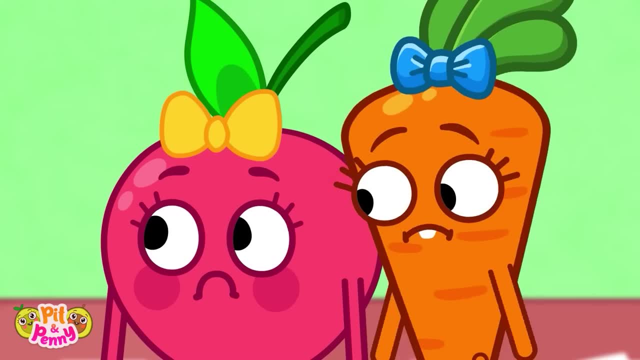 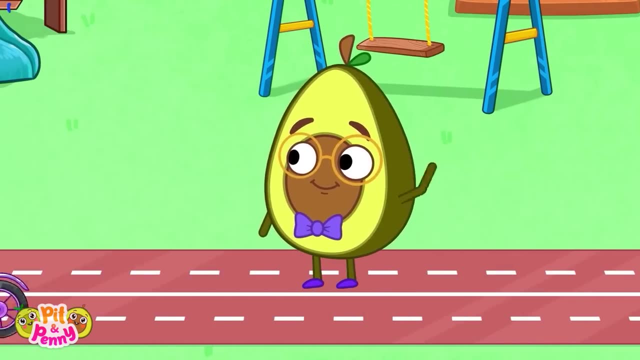 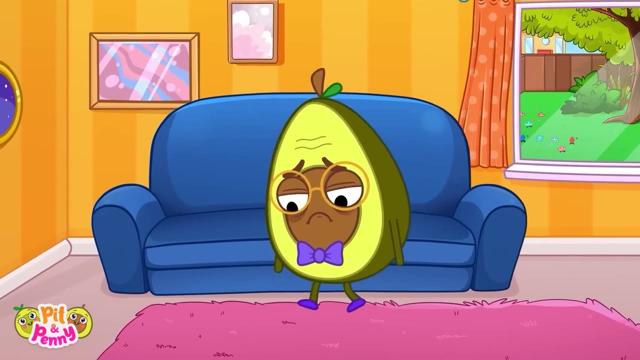 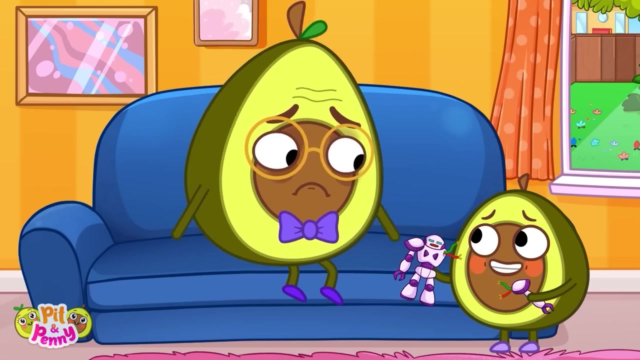 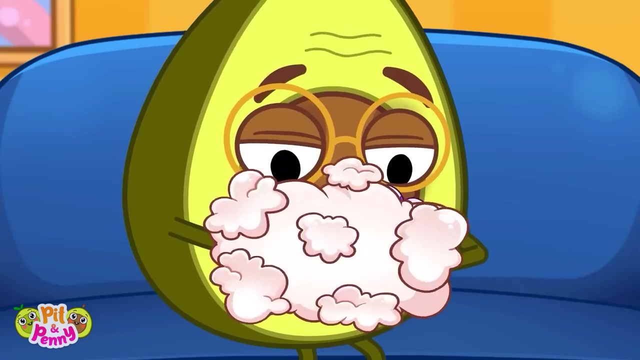 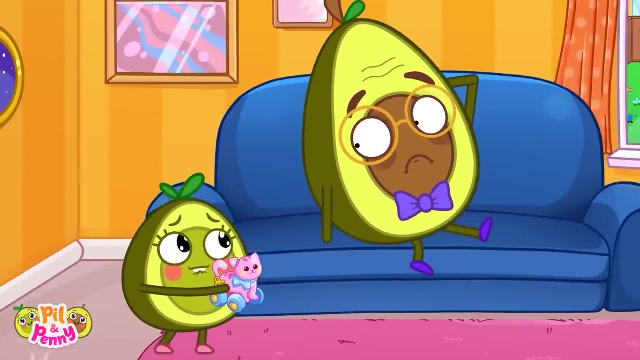 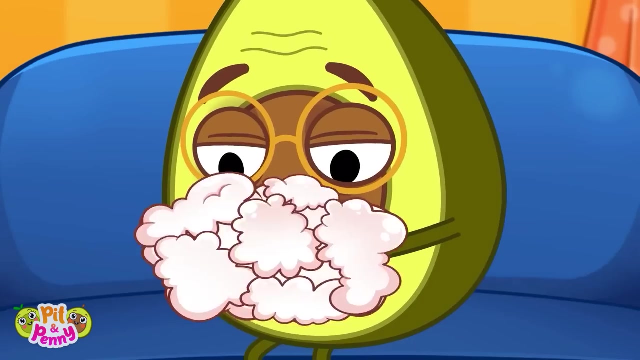 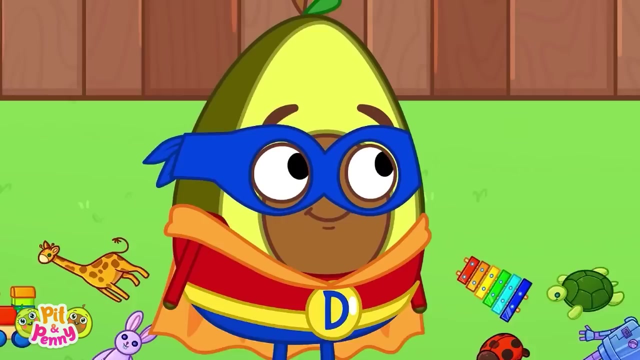 There Good as new. Thanks, Daddy. Now everyone can be friends. Finally Daddy can relax. First, Pit needs his robot fixed- Okay, And Penny needs her kitten fixed Okay. Shh, Daddy is asleep. Careful, Penny, Those pieces could fall. 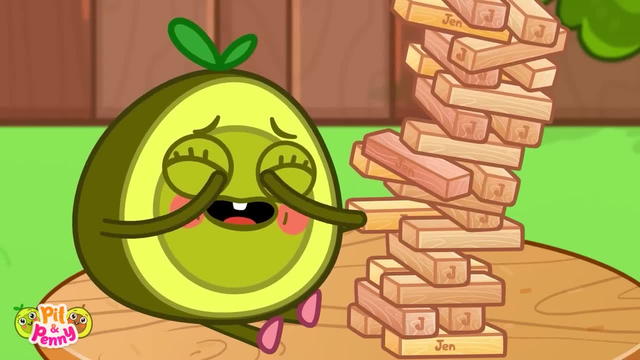 Daddy, Help me. Daddy saved Penny, Yay, But he's running out of energy. Daddy Help. Oh no, Pit might fall And the branch is breaking. Daddy saved Pit, But now Daddy is tired. Daddy Penny's stuck in the tree. 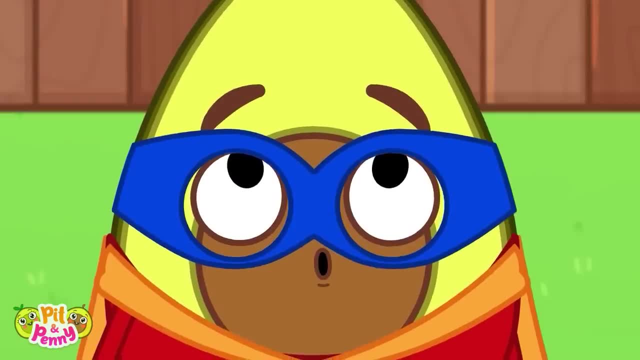 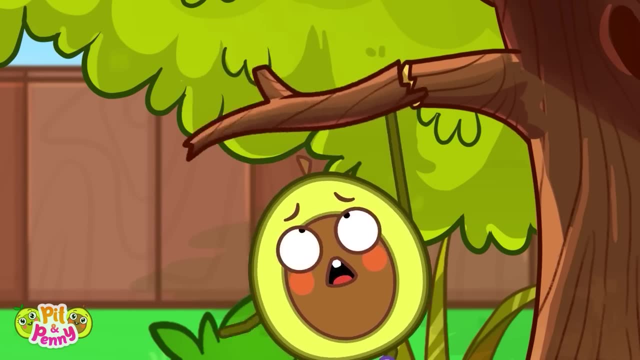 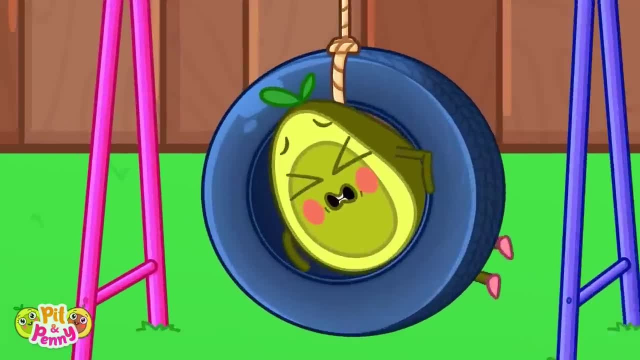 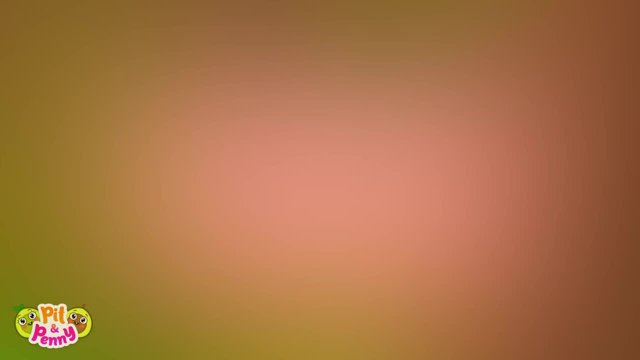 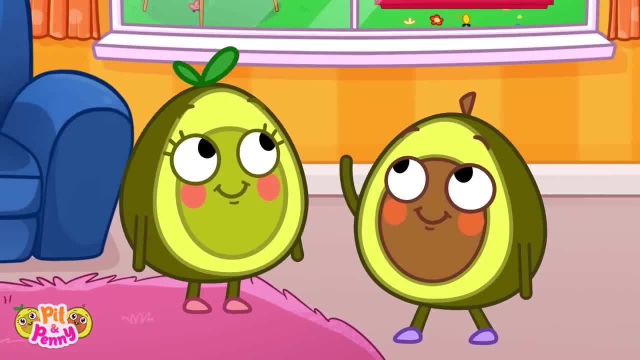 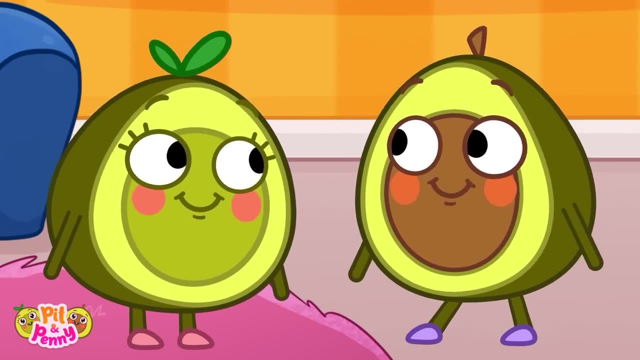 Ow, Ow, Ow, Ow, Whup, Ahh, Wup. Sadly, I lost to Patty just before I realized she was just as Raspy, asia, Oh no, Oh, no, No, Oh, no. Poor Daddy has no more energy. 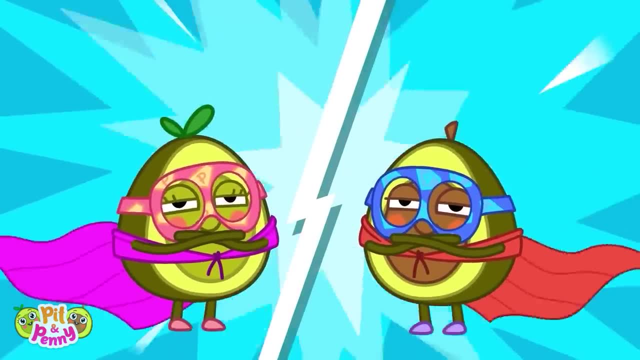 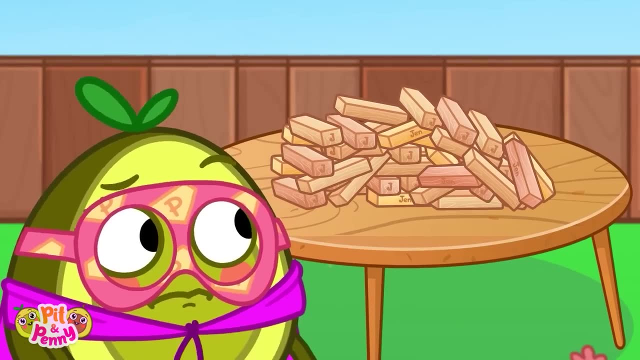 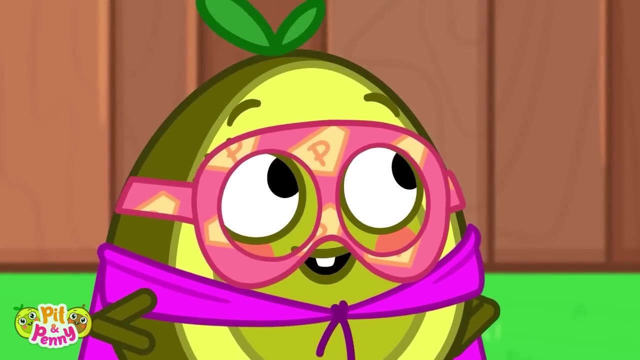 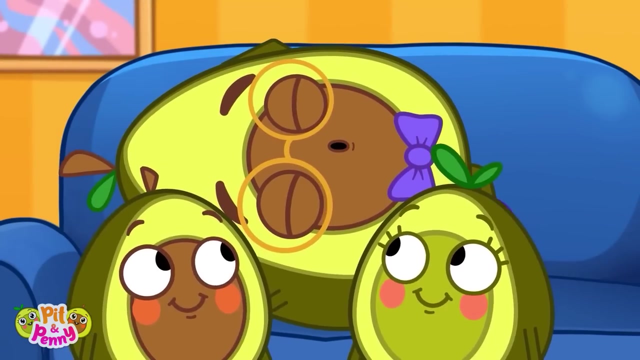 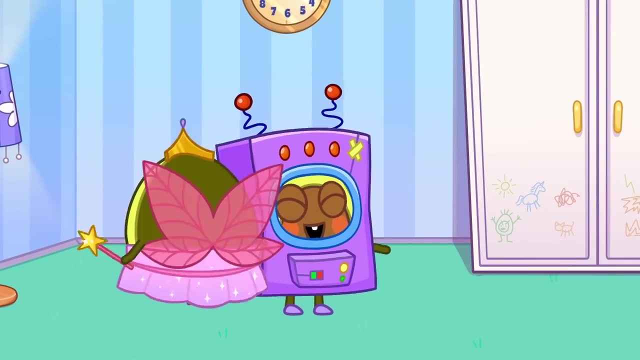 Oops, Shh. Maybe you kids can clean up this mess. Let's start with cleaning the toys. Put those wood blocks back in place And tidy the sandbox. Then kiss Daddy while he sleeps. Pit and Penny are having fun playing dress-up. 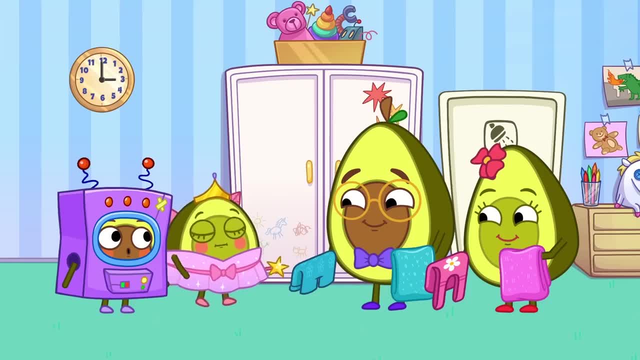 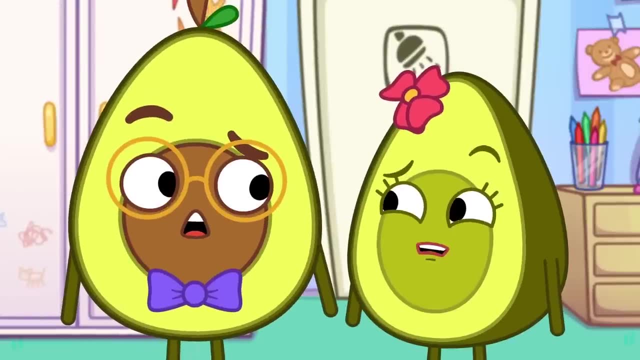 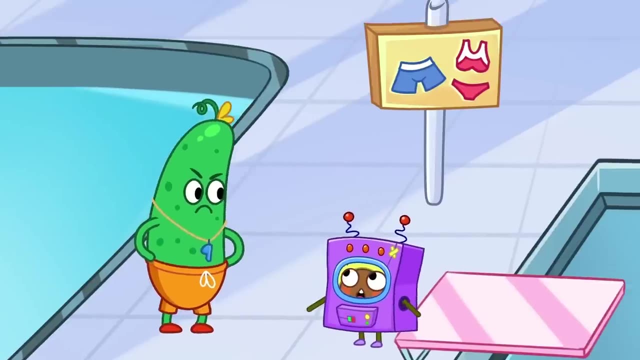 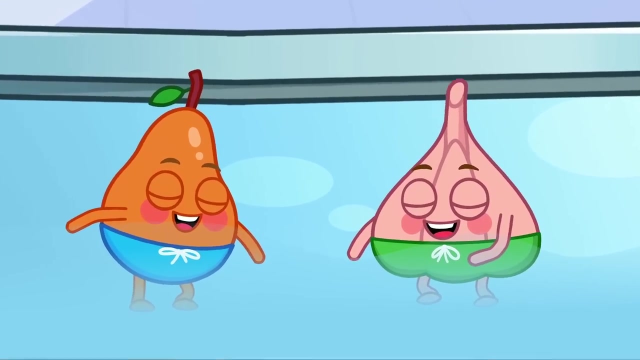 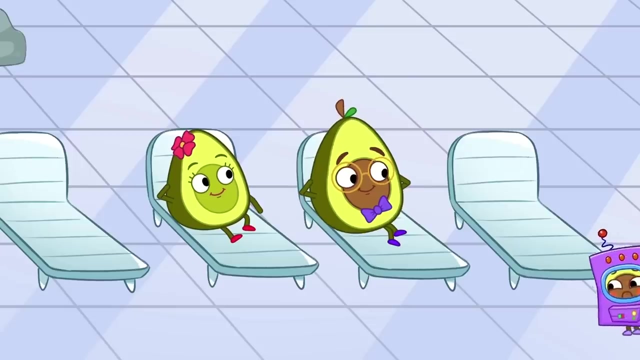 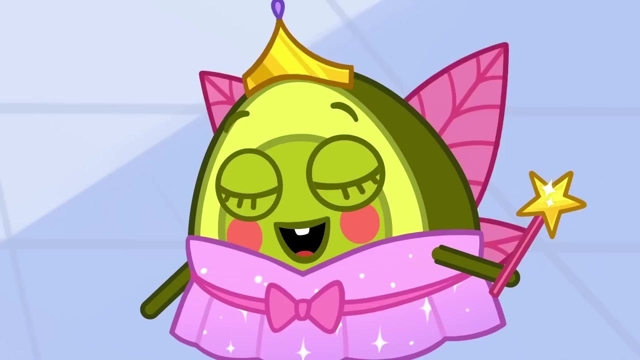 But it's time to go swimming. Don't forget your bathing suits. Oh Pit, You can't wear your robot costume in the pool. You need your bathing suit. Poor Pit Penny loves jumping off the high dive platform. Wait, Penny. 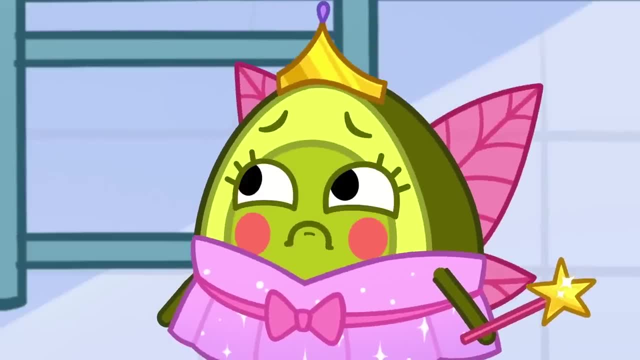 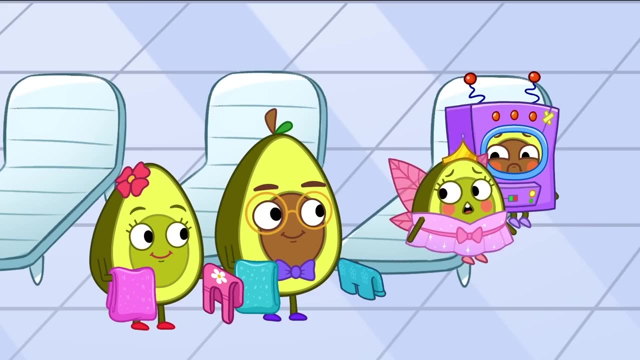 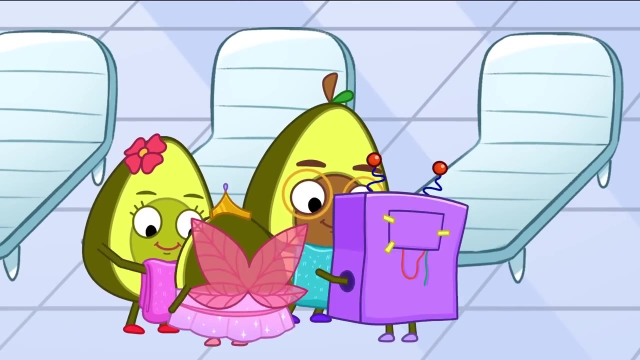 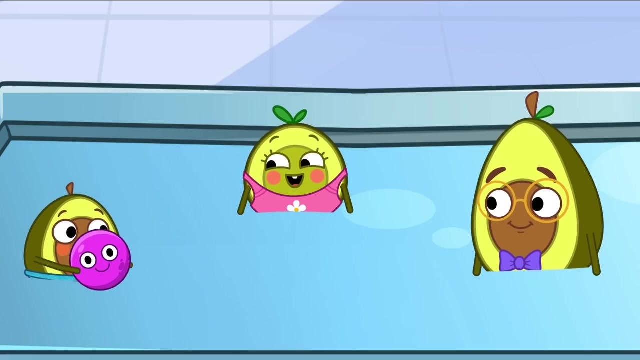 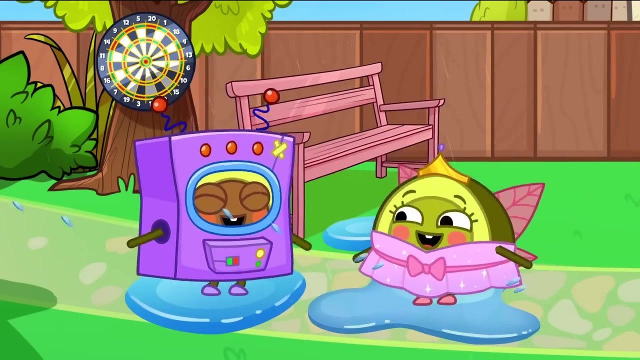 You can't wear your fairy costume in the pool, Poor Penny. Look what Mommy and Daddy brought. Thank you, Mommy and Daddy. It's raining outside. Playing in puddles can be lots of fun, But now Penny's costume is muddy. 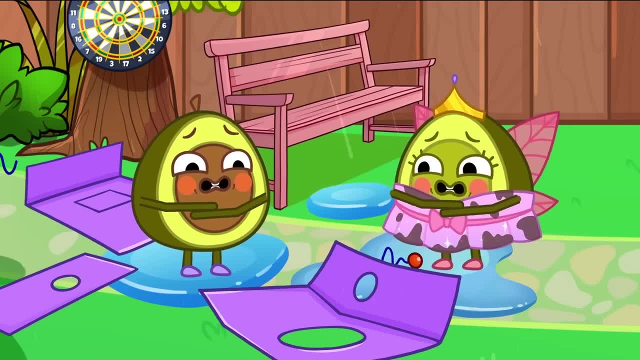 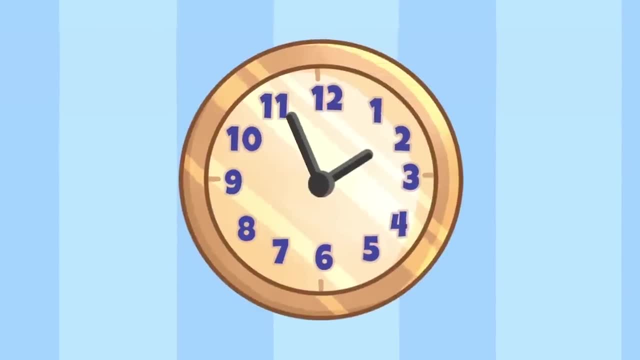 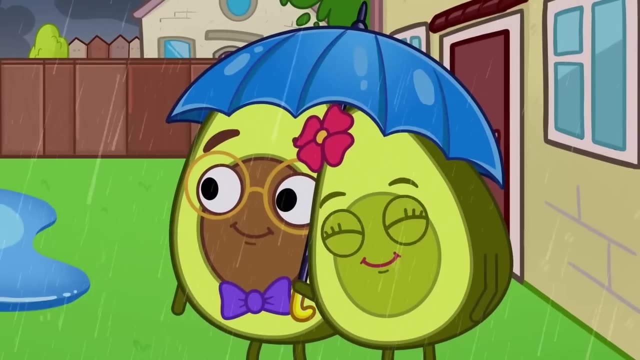 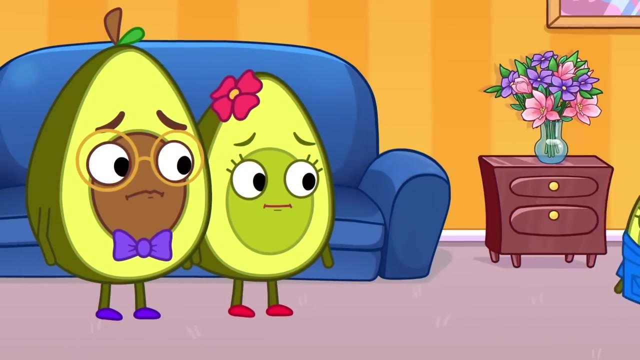 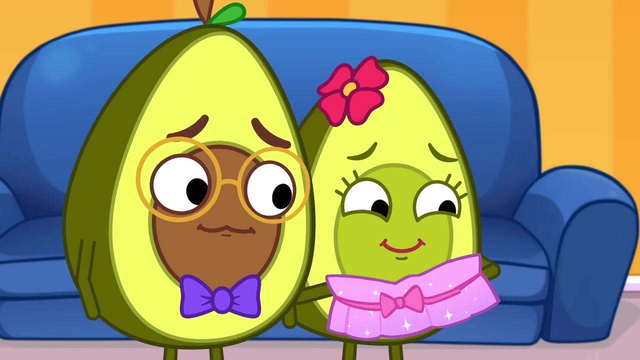 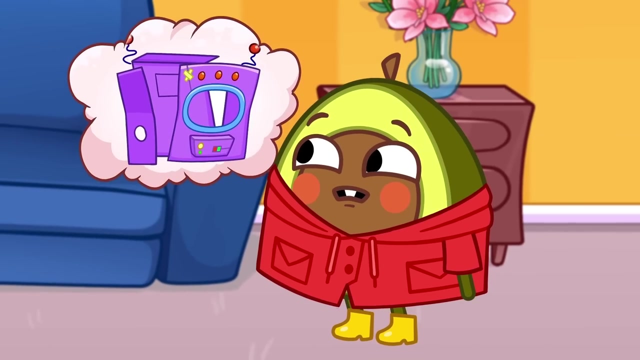 And Pit's costume is broken. Huh, Huh, Hmm. Okay, Raincoats and rubber boots are a much better choice. Oh-ho, Penny wants to play in her fairy costume- Mom washed it. And Pit wants to play in his robot costume. 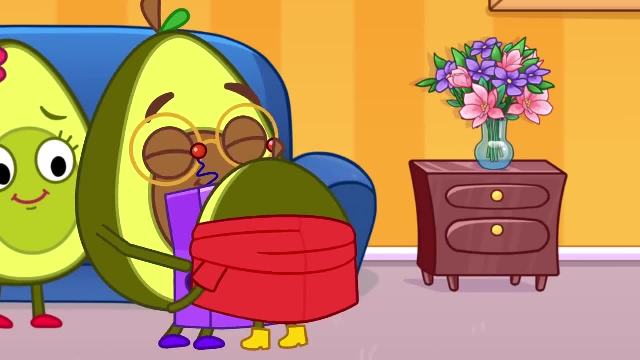 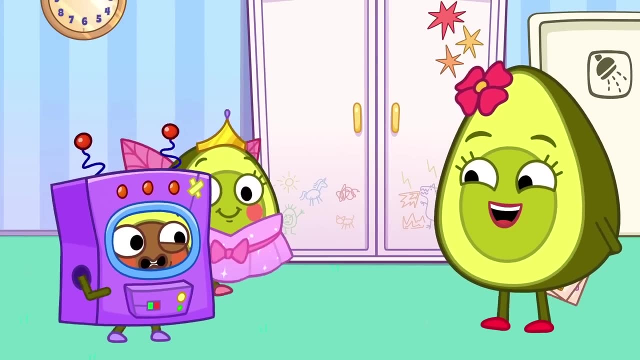 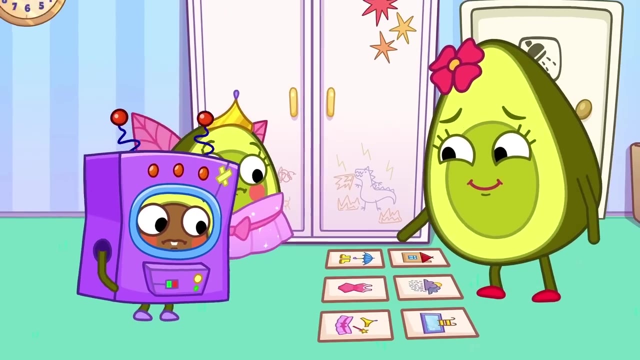 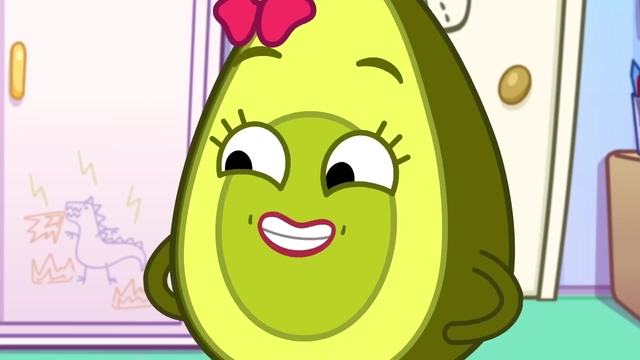 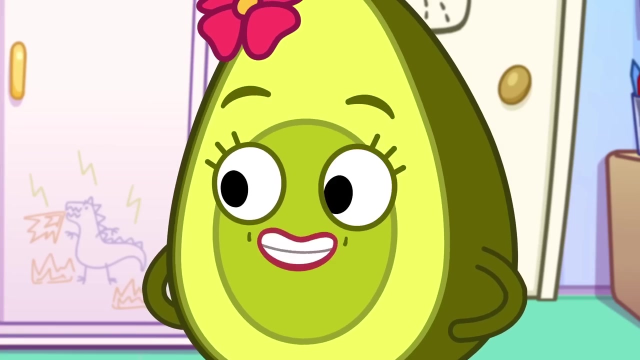 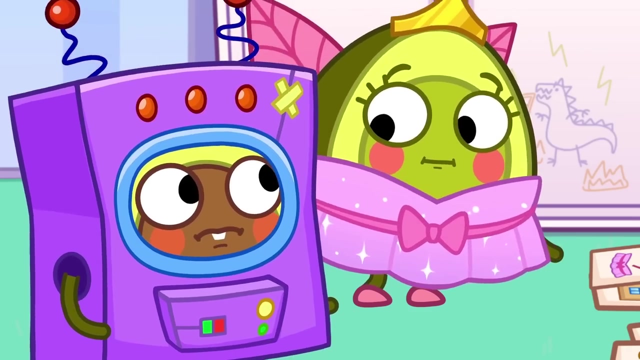 Dad fixed it. Let's see what Pit and Penny learned today. What outfit can you wear at home? Costumes can be worn at home. And what do you wear when it rains? Rubber boots and rain gear, Right, Yay, And that means you wear a bathing suit at the pool. 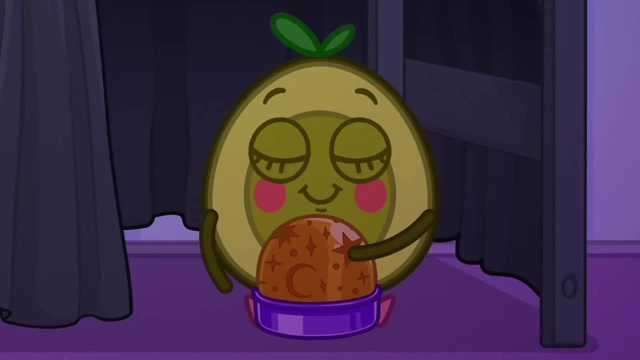 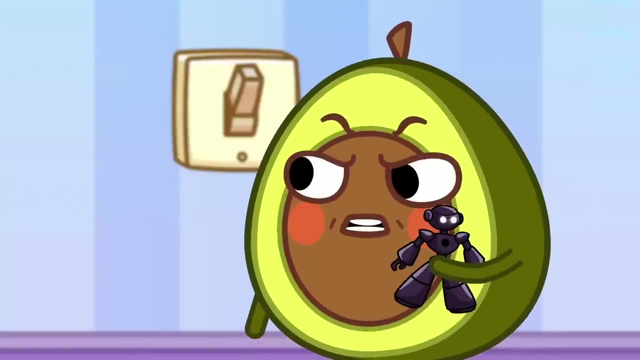 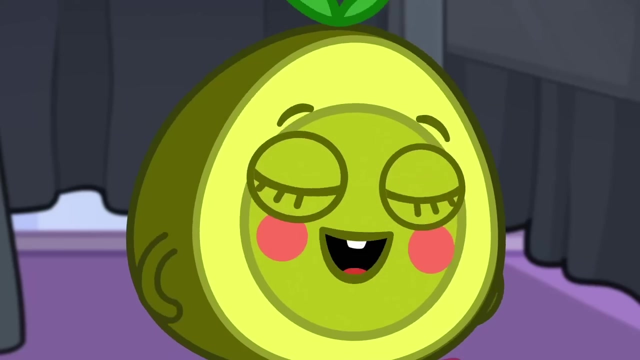 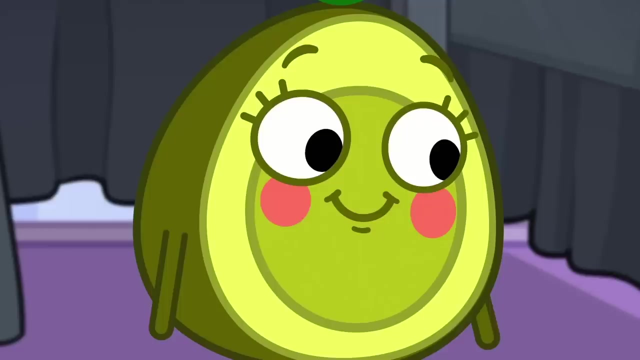 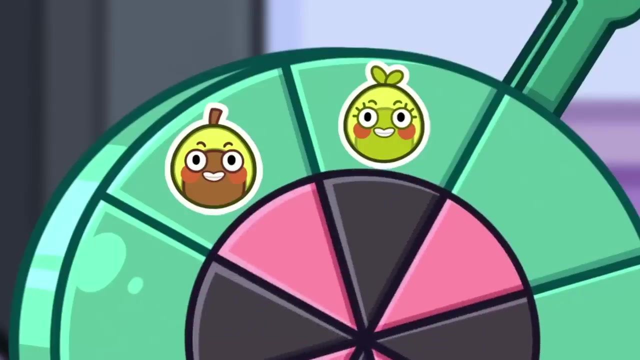 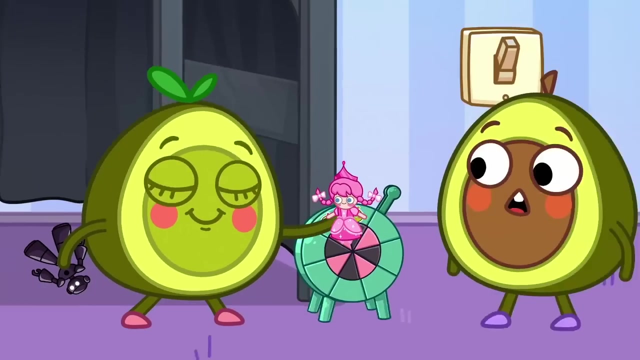 Good job. Penny has set up a cool fort to play in. Black is my color. The color picker will choose your color. Let's check it out. Pit landed on pink. Pink again. Penny gets the black toys And Pit gets the pink ones. 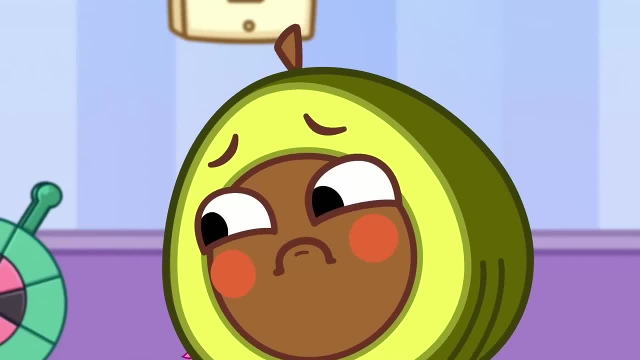 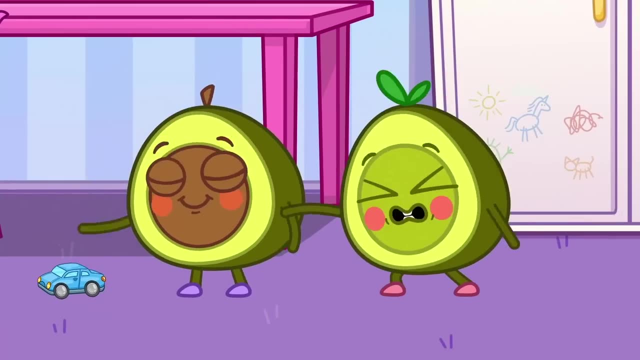 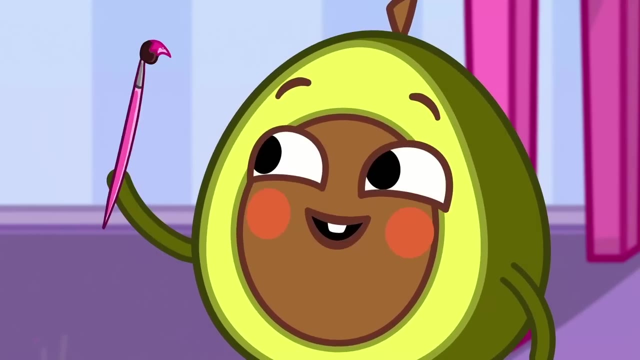 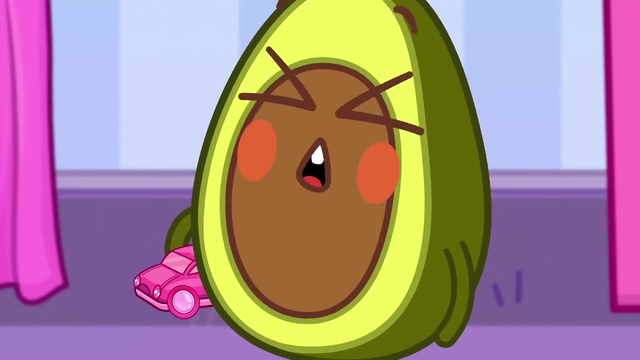 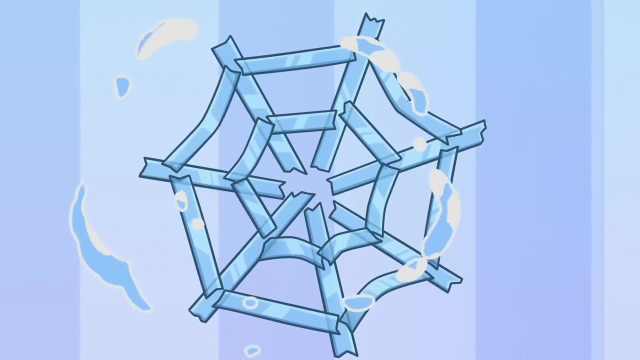 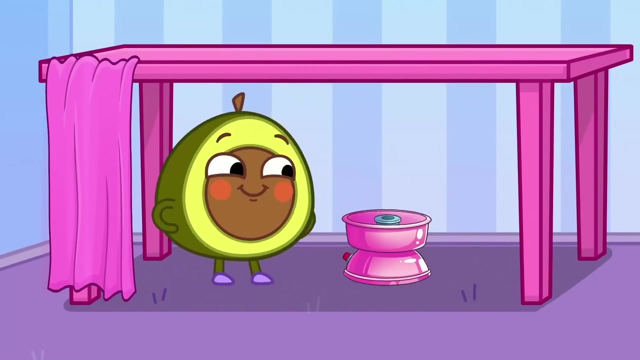 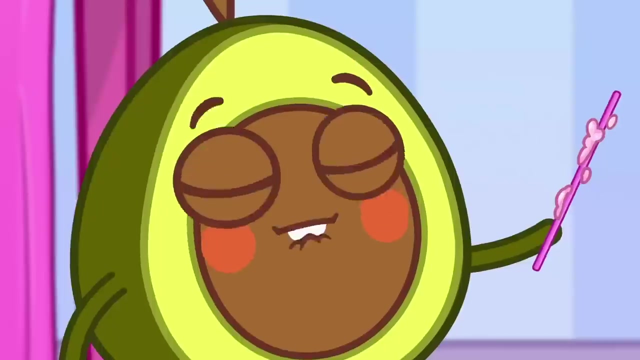 There's even a pink fort for Pit. Sorry, Pit, You can only play with pink cars There. Now he can play with the pink car. Whoa, Penny made a surprise Spiderweb And Pit made cotton candy. Penny has a black blow-up mattress. 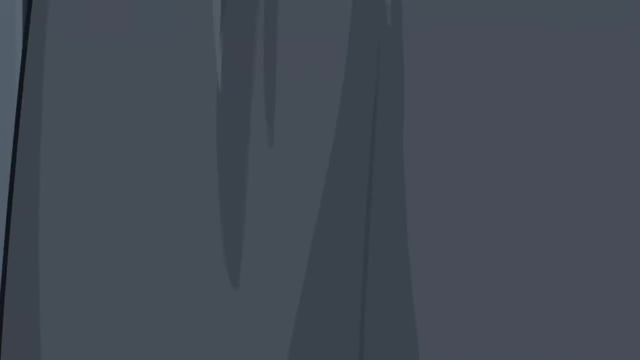 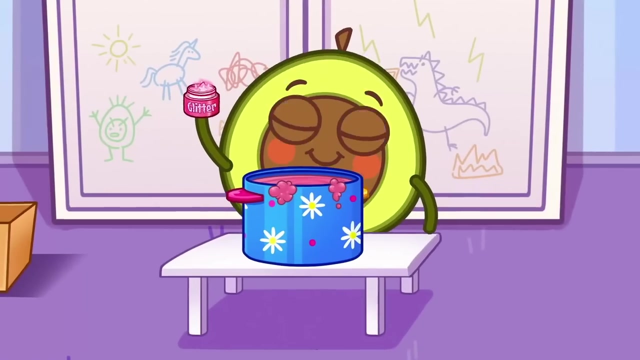 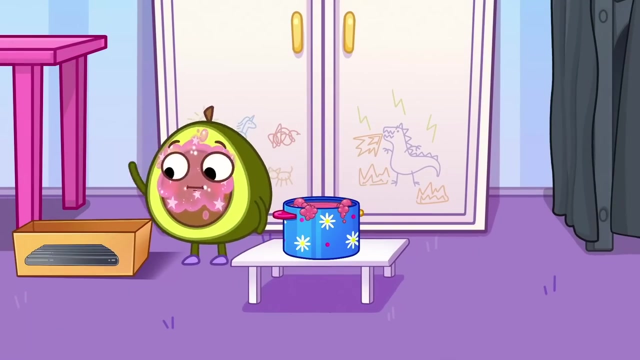 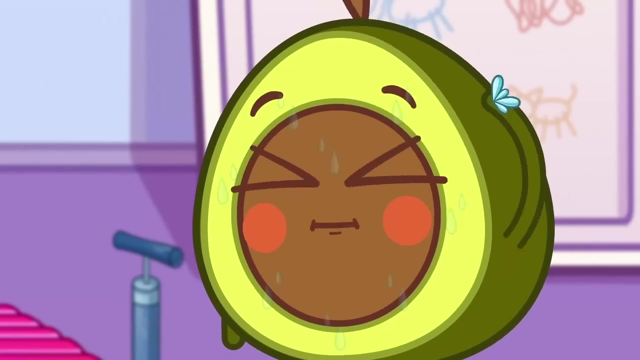 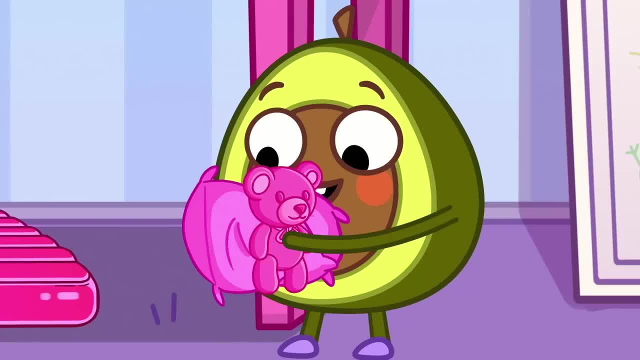 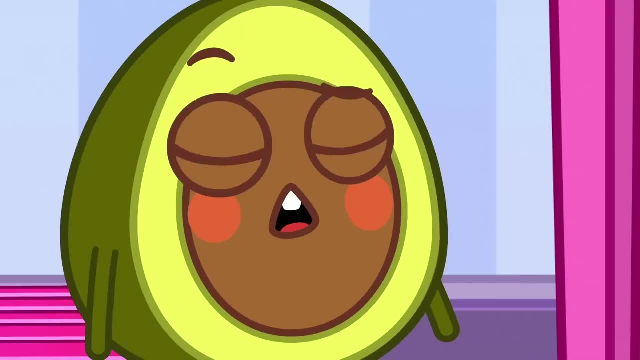 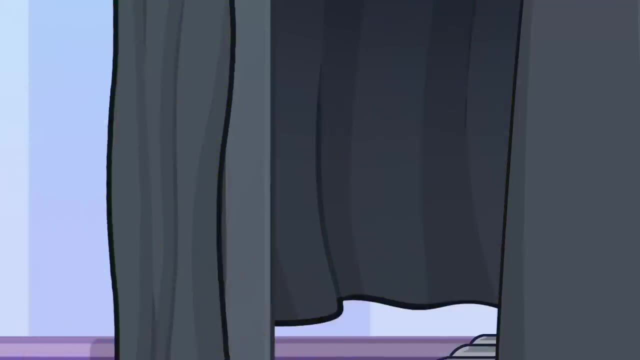 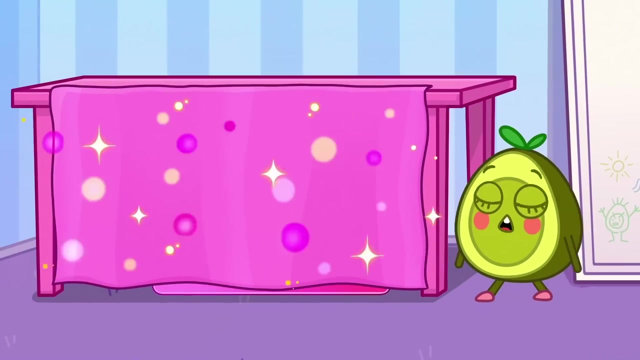 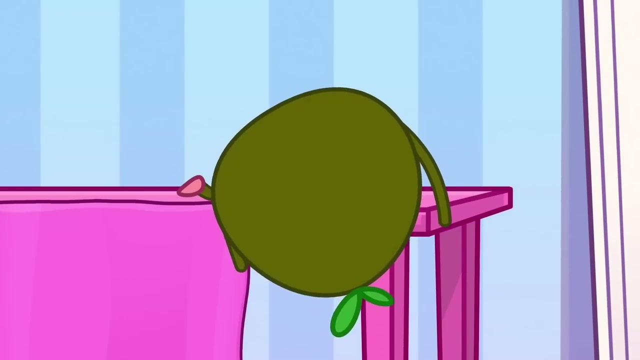 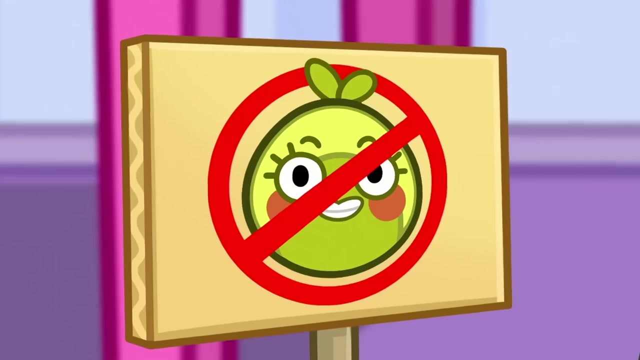 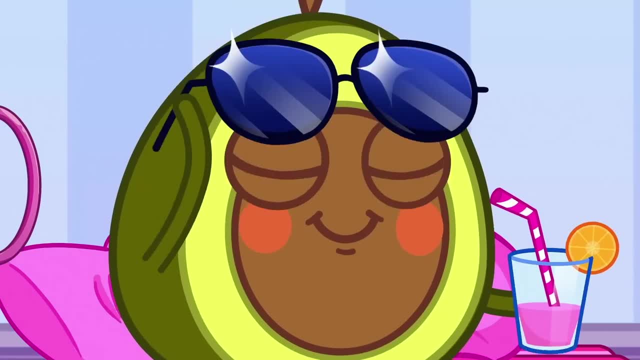 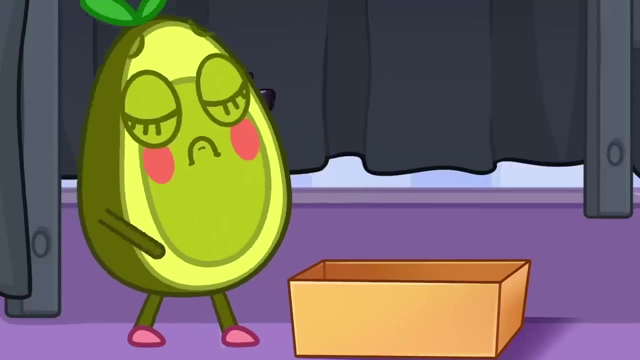 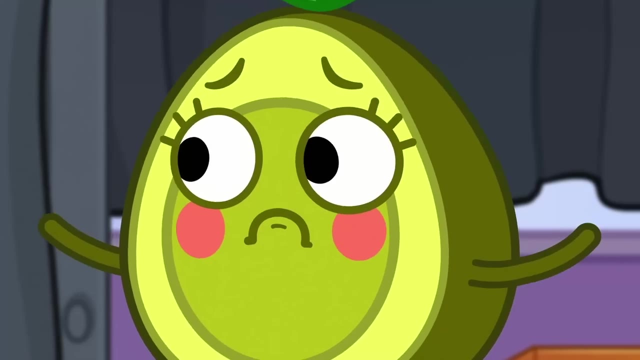 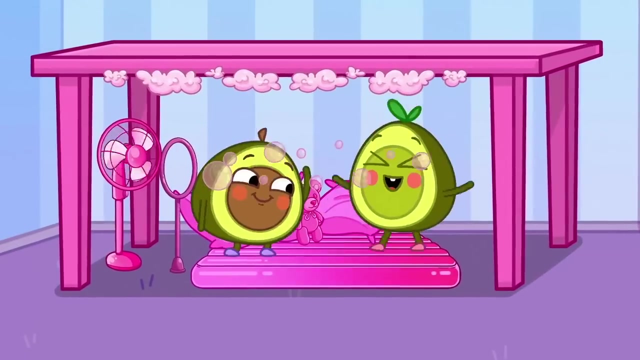 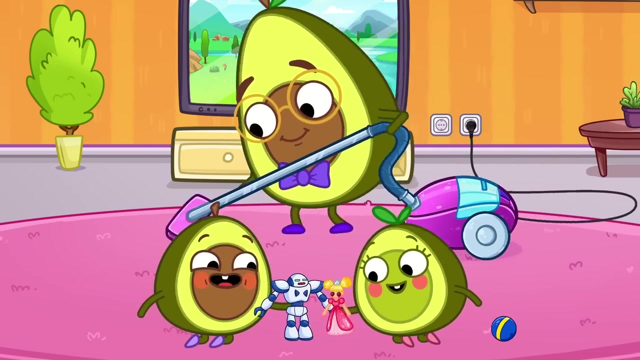 Penny's not having fun anymore. Your secret room is better. Let's play together. What a great idea, Pit. Now you'll have even more fun. Pit and Penny are having fun. Penny and Penny are playing while Mommy and Daddy clean. 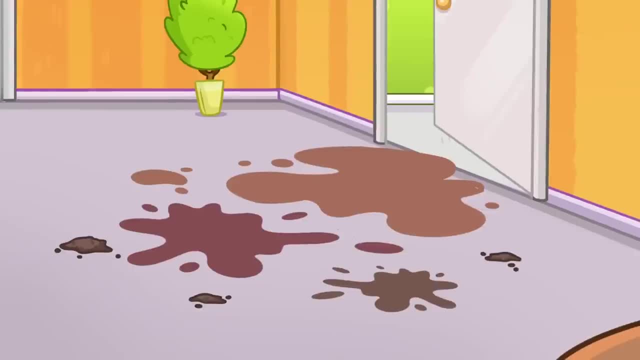 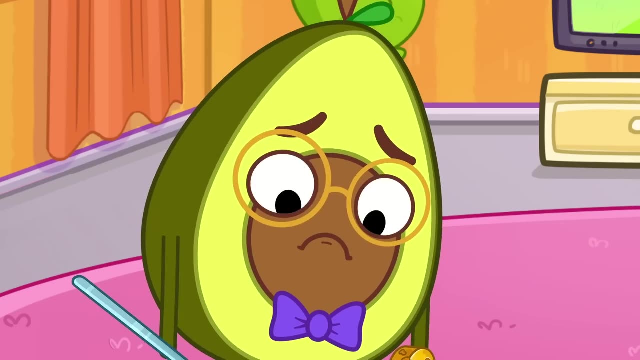 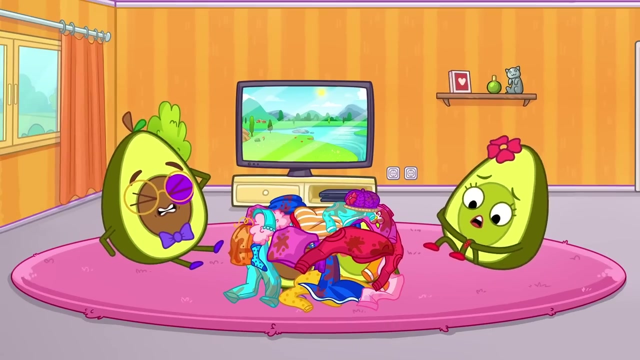 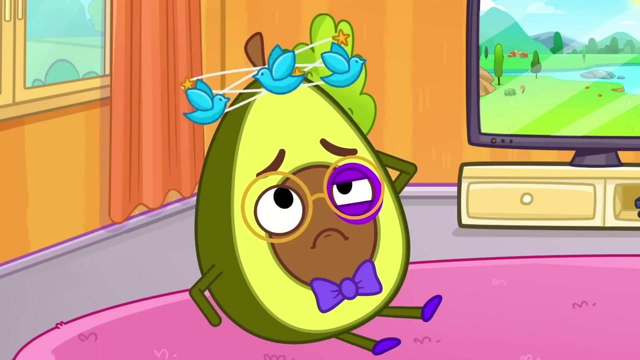 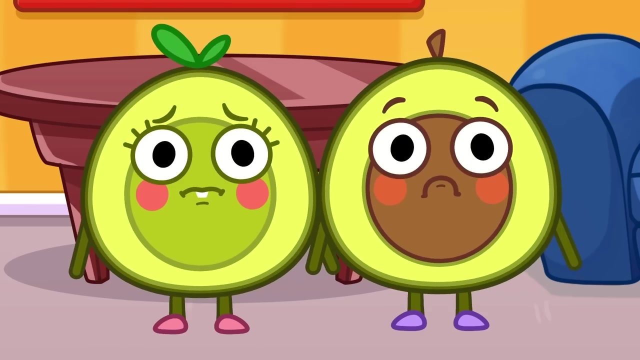 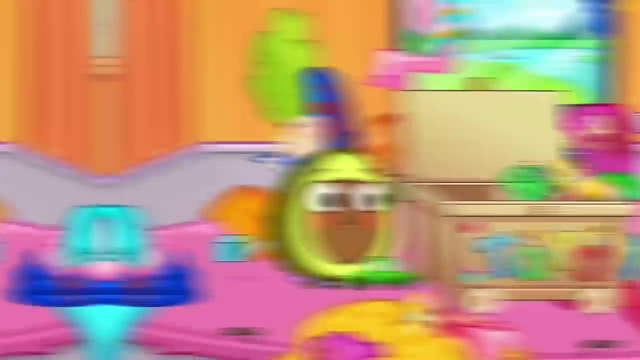 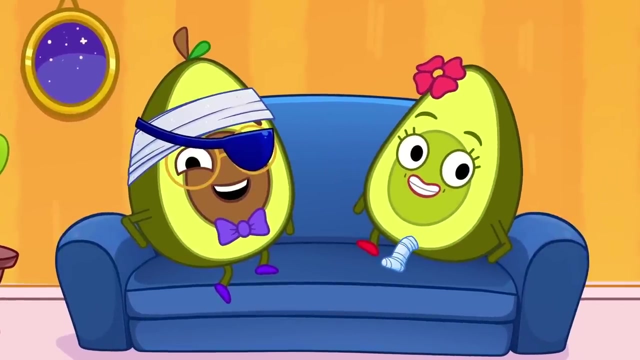 Sorry, kids, but you have chores too. Mommy hurt her knee And Daddy Daddy hurt his head. Now you have to do all the work, kids, It's easy to put your toys away. Huh, Huh, Ta-da, Ta-da. 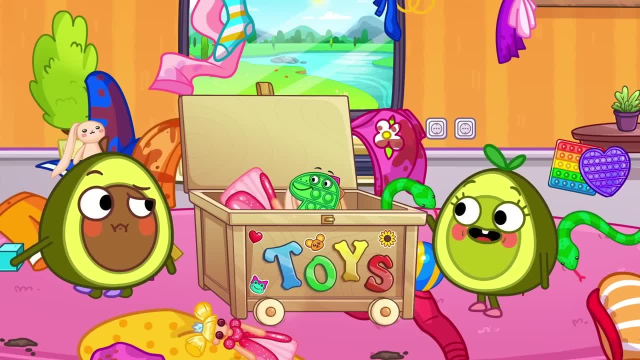 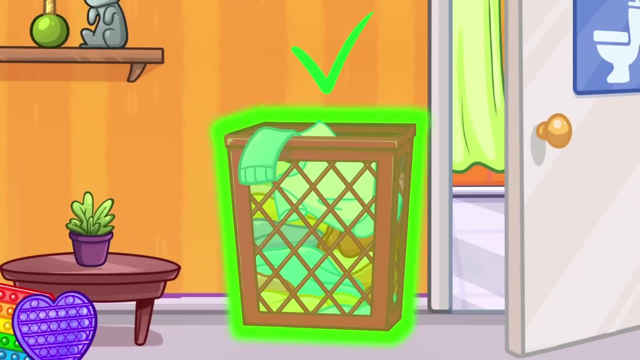 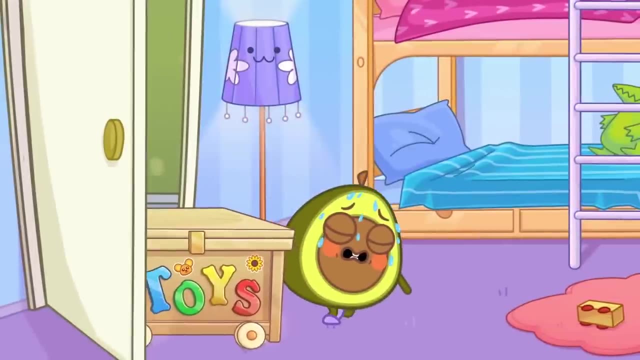 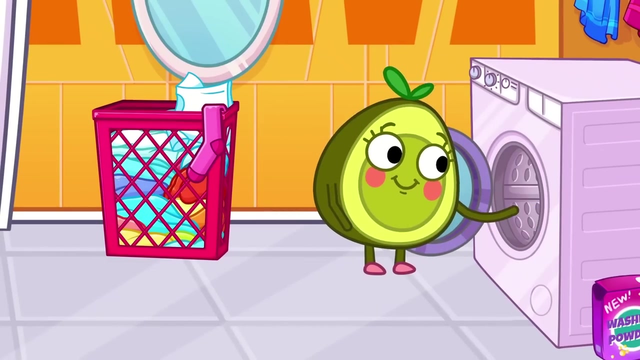 Whoa, Huh, Huh, Huh, Huh, Huh, Huh Huh. Clothes don't go into the toy box, They go in the hamper. Penny's doing laundry. You're doing laundry, Ta-da. 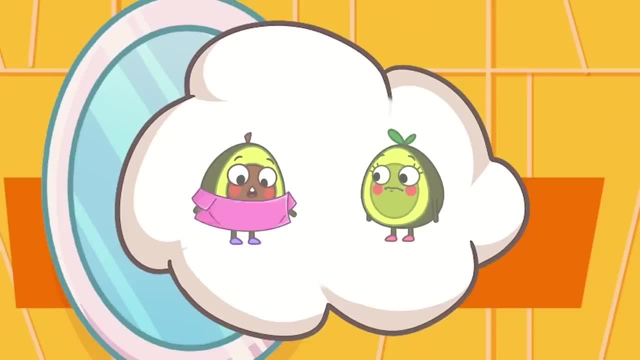 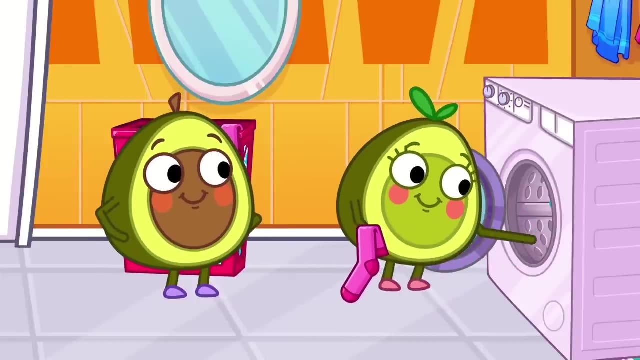 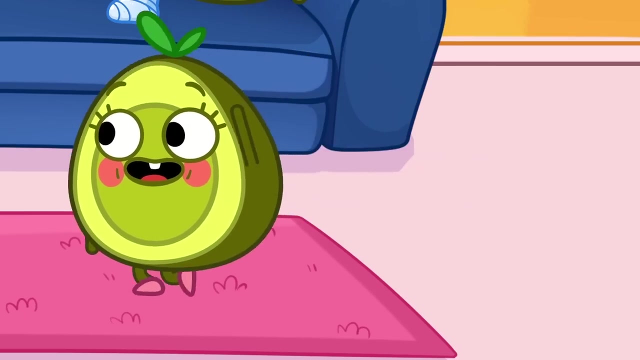 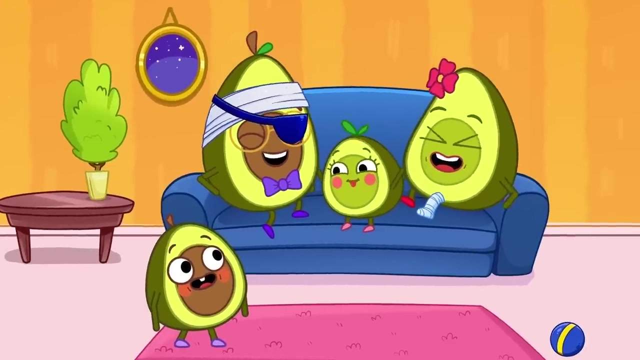 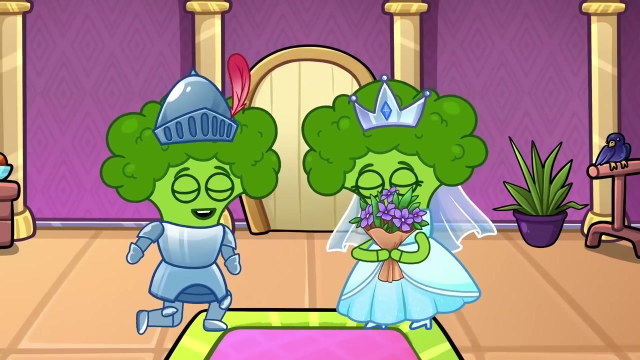 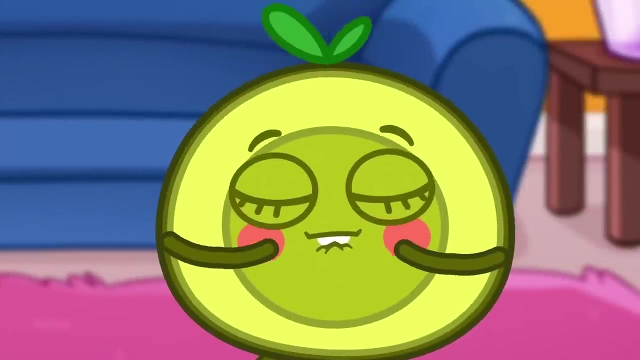 Ta-da, Huh Huh. You can't wash whites and pinks at the same time. The chores are all done. Now it's time for fun. Pit and Penny are watching a movie, But it's almost bedtime. You can finish watching it tomorrow. 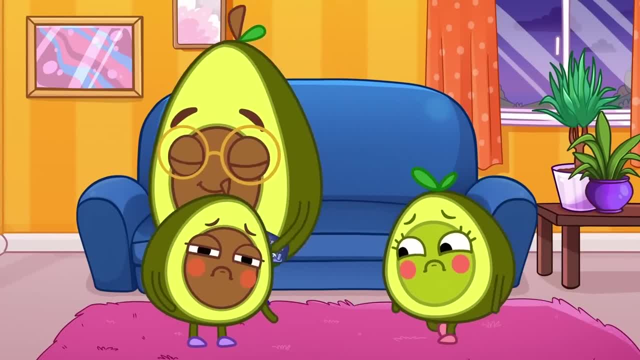 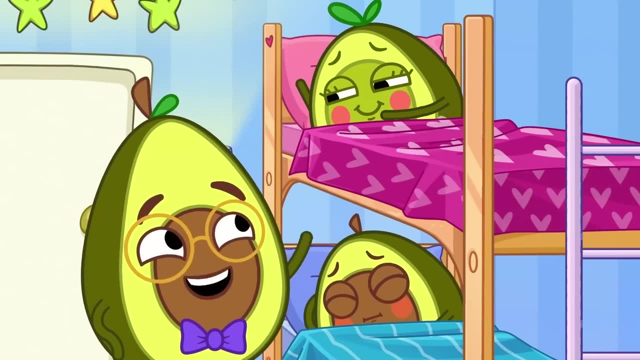 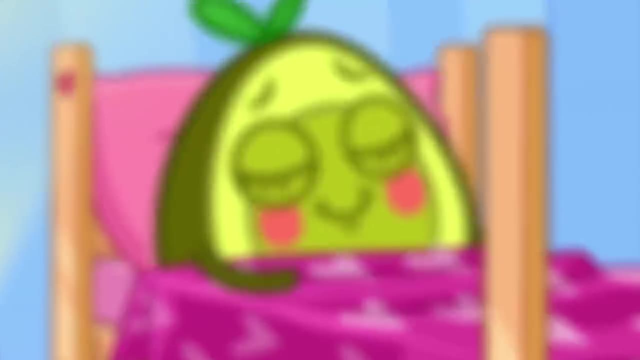 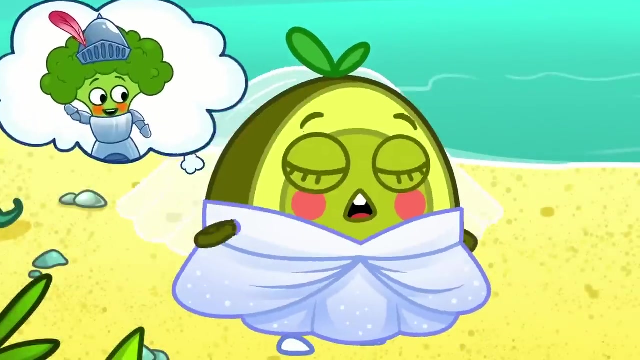 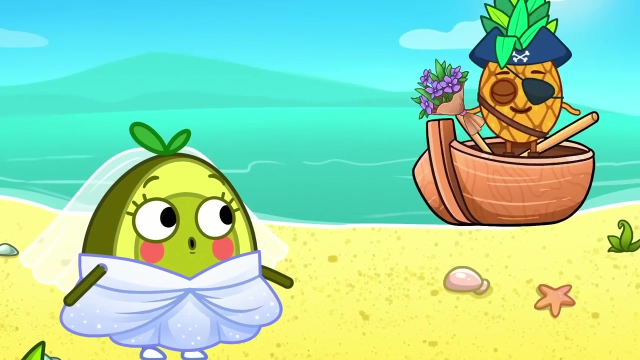 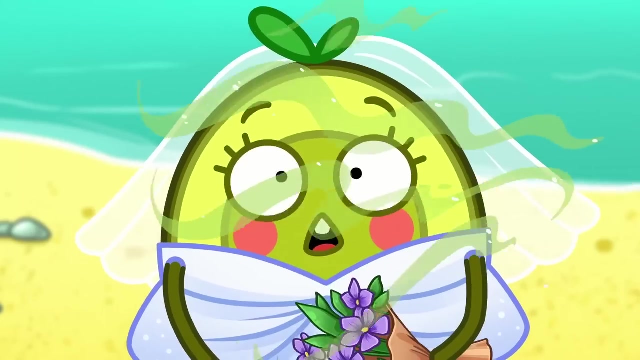 It's time to sleep, kids. Good night, kids. Penny dreams she is wearing a wedding dress. Who can she marry? Maybe she can marry Captain Pineapple the pirate. What is that awful smell? Maybe Captain Pirate isn't the one. 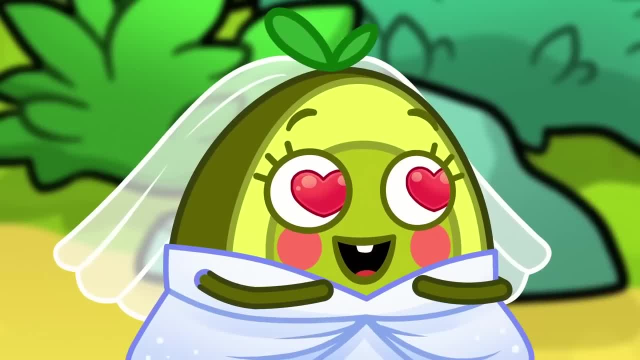 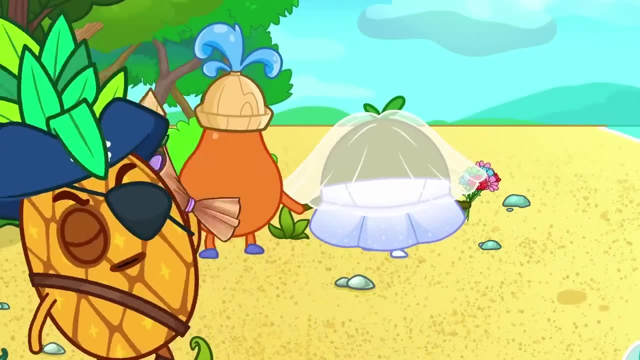 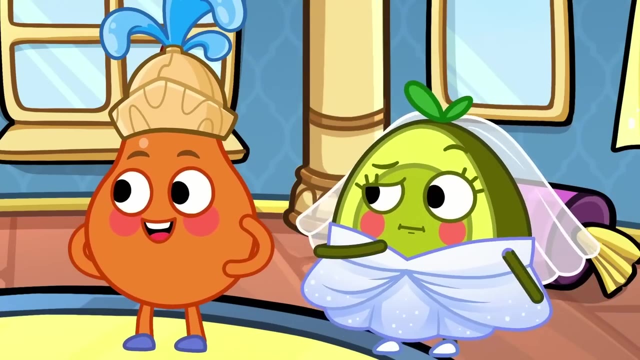 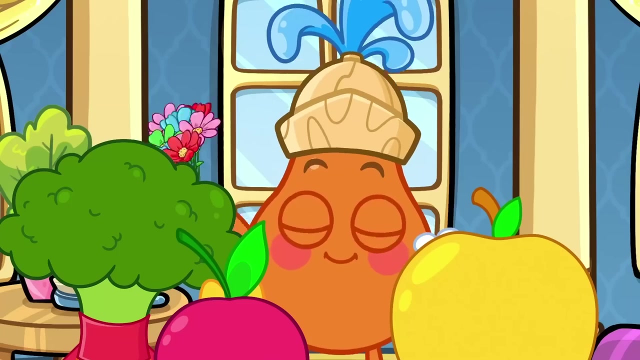 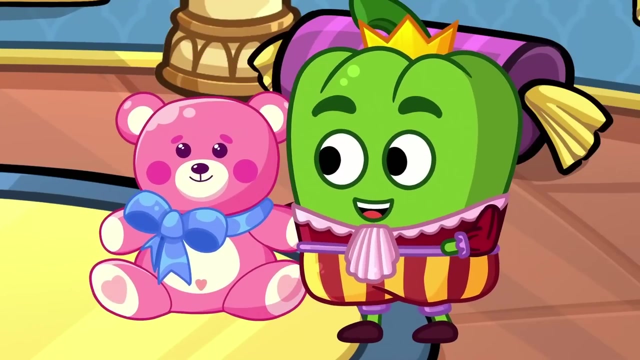 Hey Penny, Maybe she can marry Sir Pear the knight. Sorry, Captain Pineapple, This is Sir Pear's home And these are Sir Pear's adoring fans. Maybe Sir Pear isn't the one. Hey Penny, Maybe she can marry Prince Pepper. 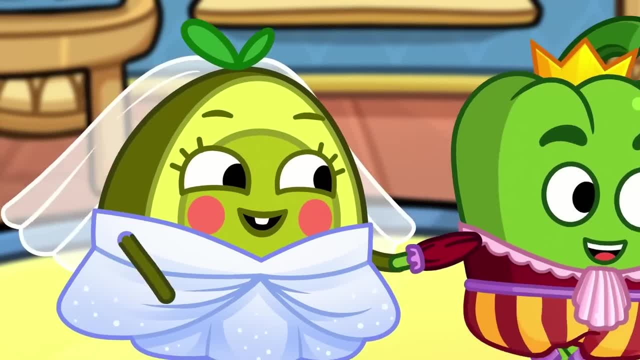 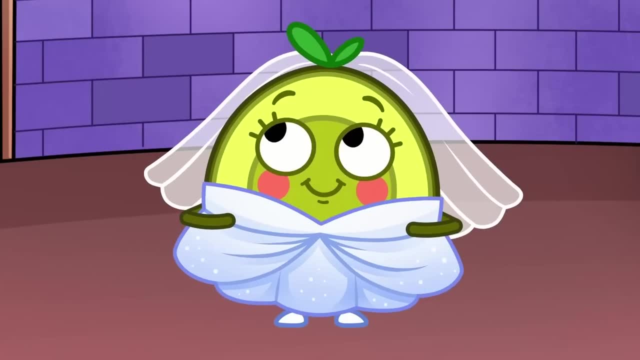 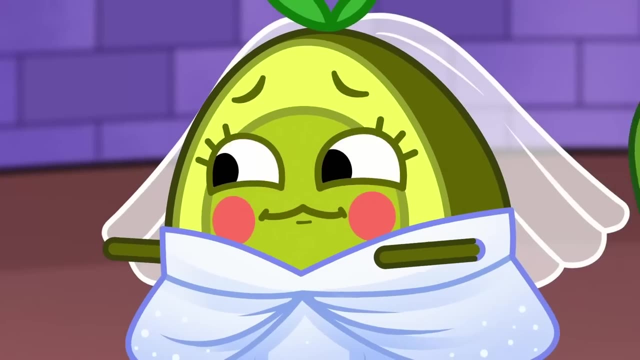 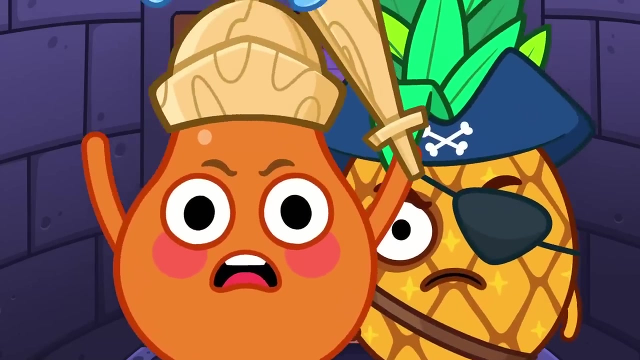 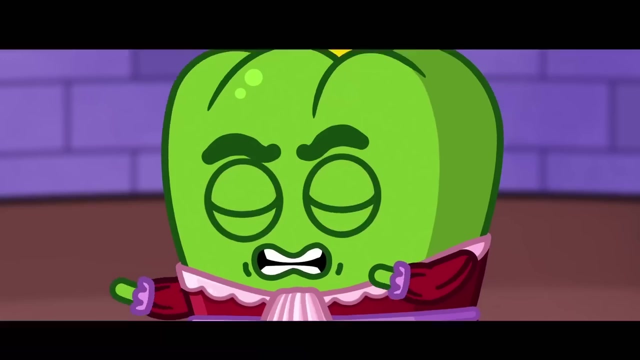 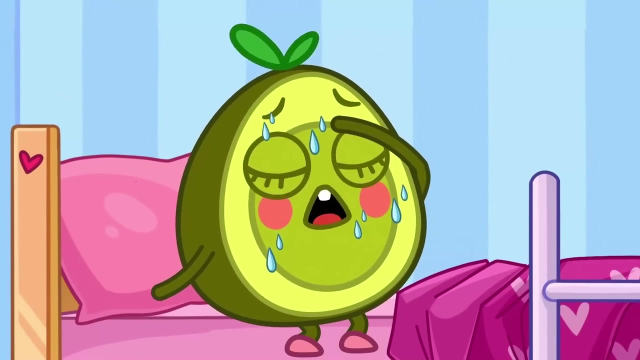 Hey, Sir Pear. Penny is the next một sankhan stepping off the boat before she gets in trouble. Sorry, Sir Pear, Watch out, Sir Pear. Oh The Всенчая. Maybe Prince Pepper isn't the one. kus, Wake up Penny. It's just a bad dream. 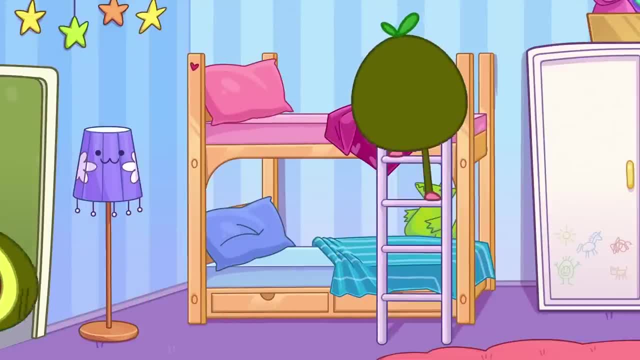 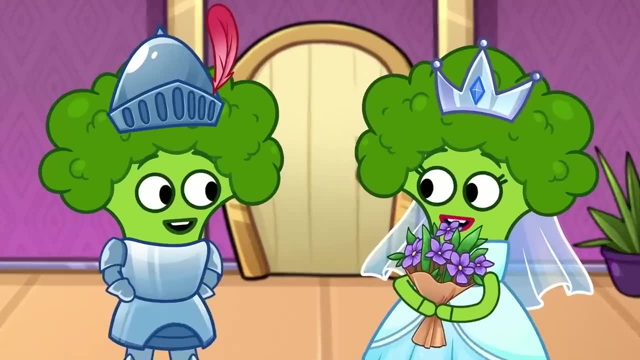 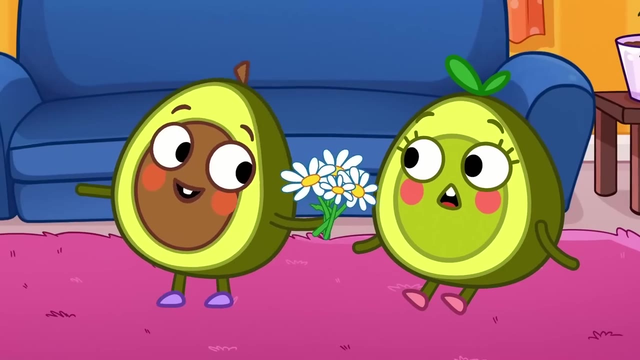 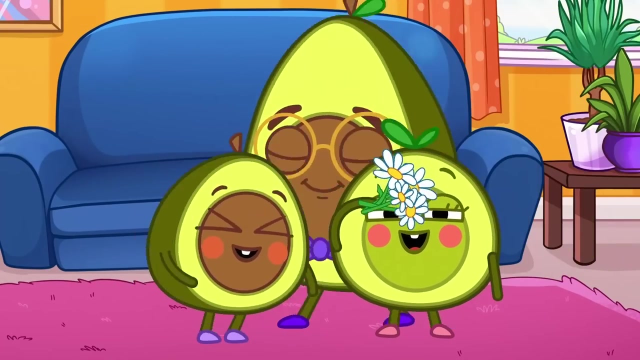 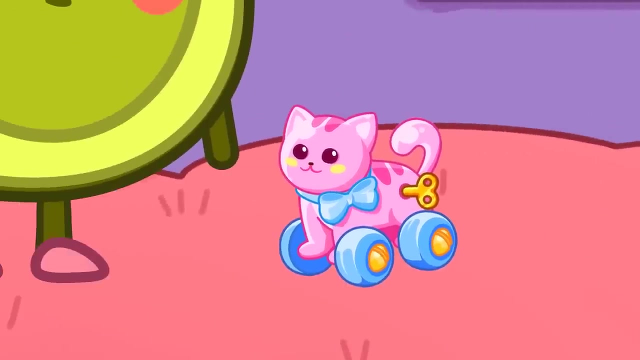 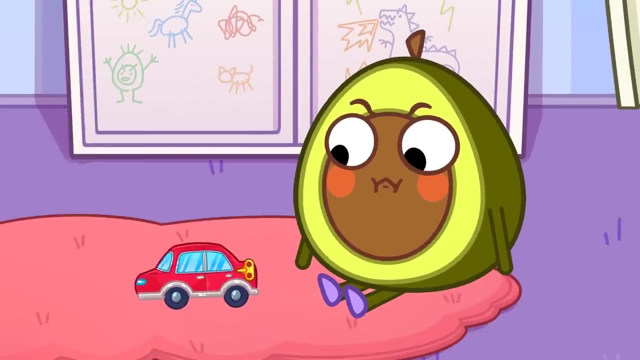 Let's watch a movie. Did you like the ending, Penny? Let's go dancing. Have fun dancing, you two. What a cute wind-up kitty cat. It's Penny's favorite toy. Pit loves his wind-up car. It might be broken, Pit. 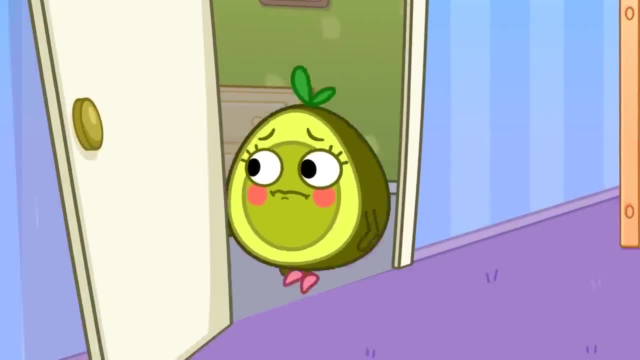 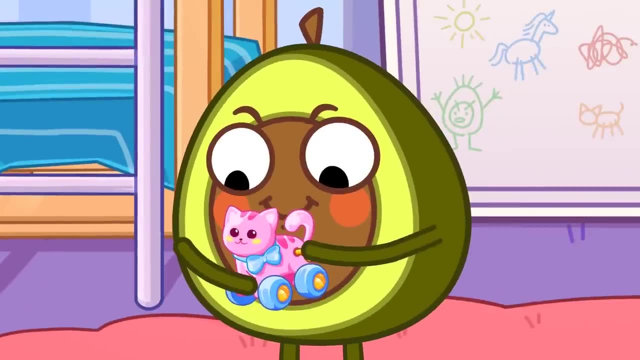 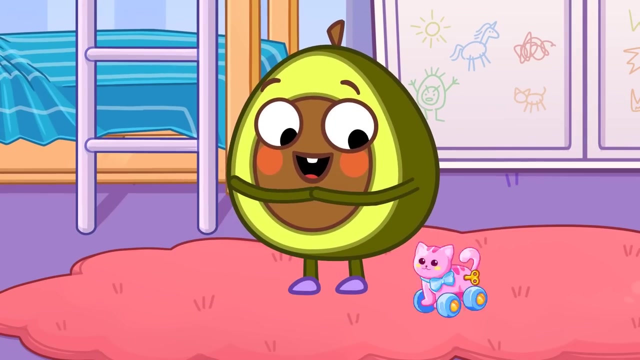 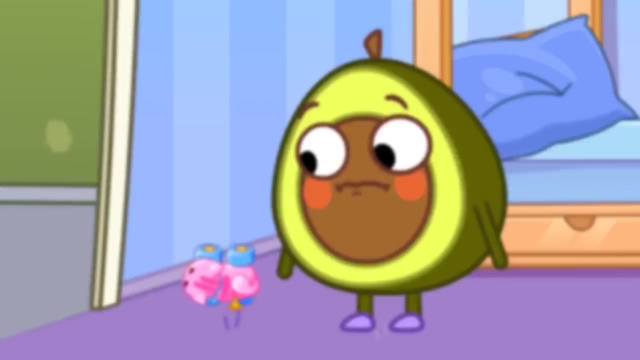 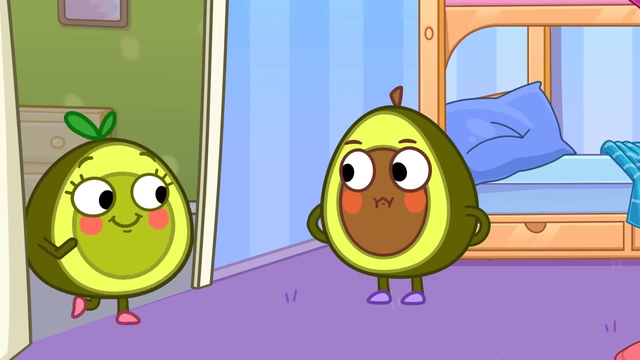 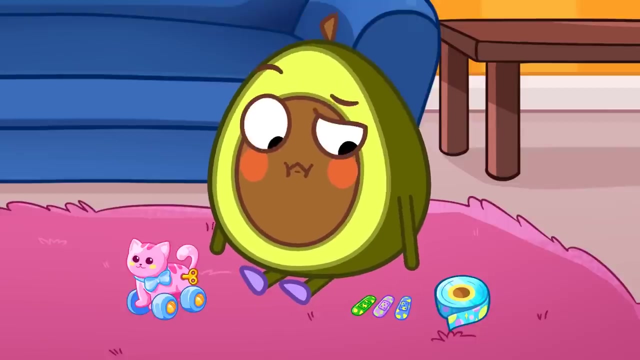 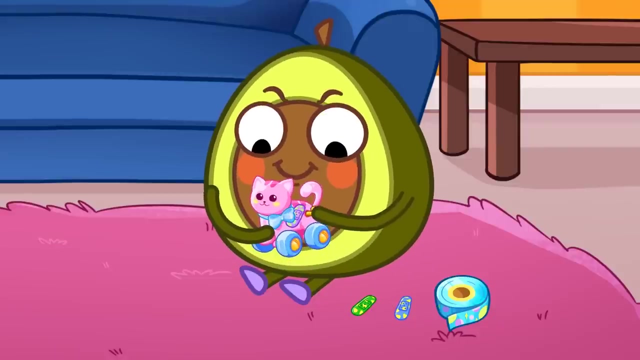 Penny needs to visit the bathroom. Don't wind it too much or it'll break. How will Penny feel now Pit decides to hide the broken toy? It's already gone. Penny, Will a bandage fix it? Nope, that didn't work. 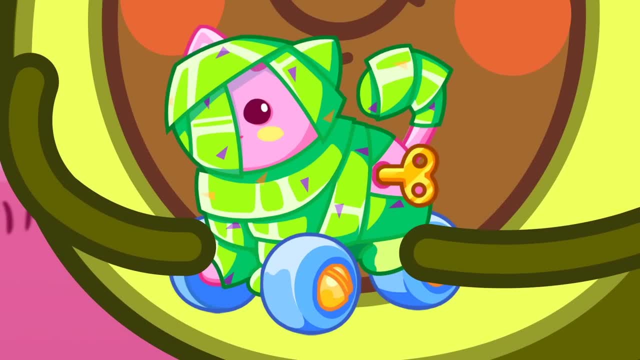 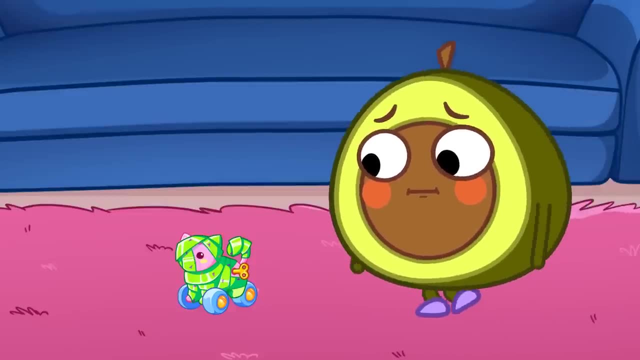 Will tape fix it? That didn't work either. What happened, Penny? You're not going anywhere. We're going to the bathroom. You can't leave me here. You're not going anywhere. You can't leave me here. You can't leave me here. 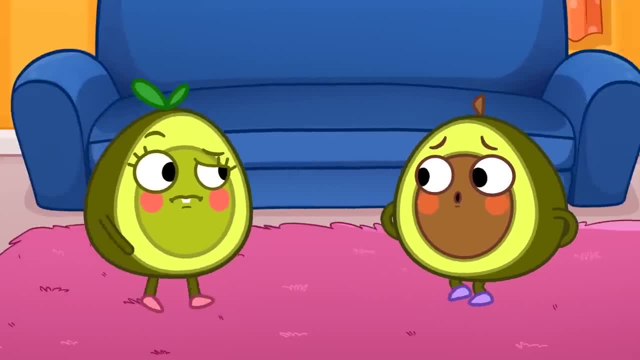 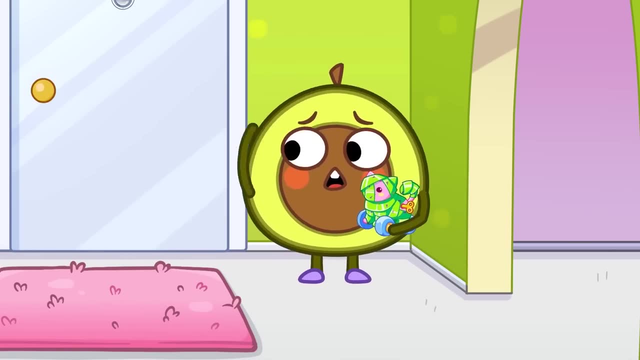 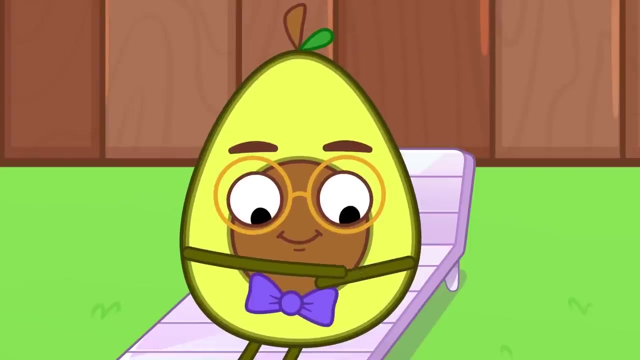 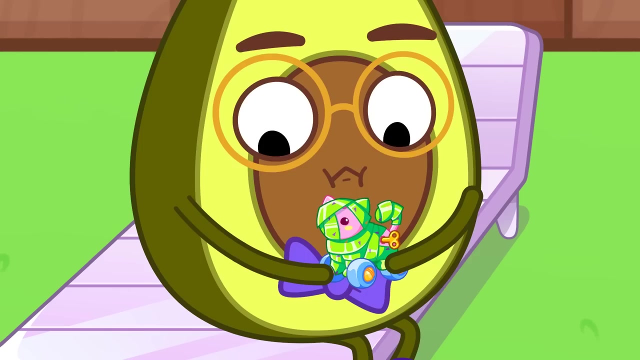 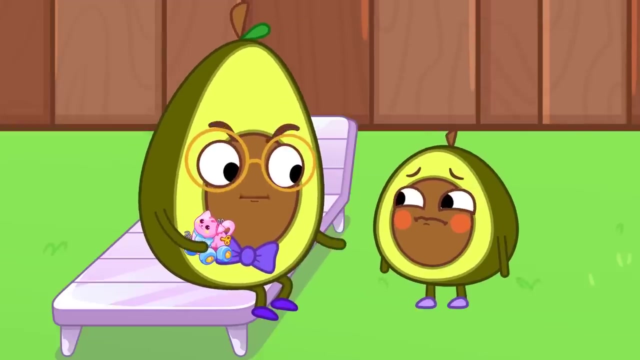 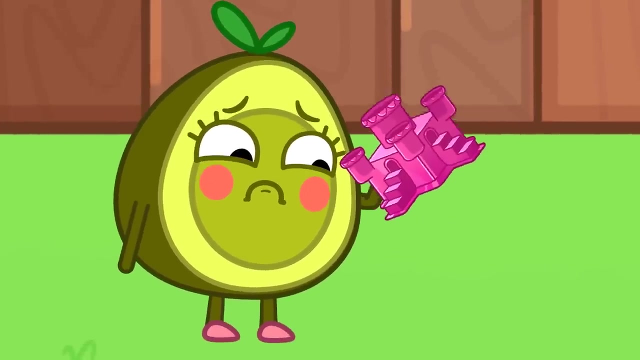 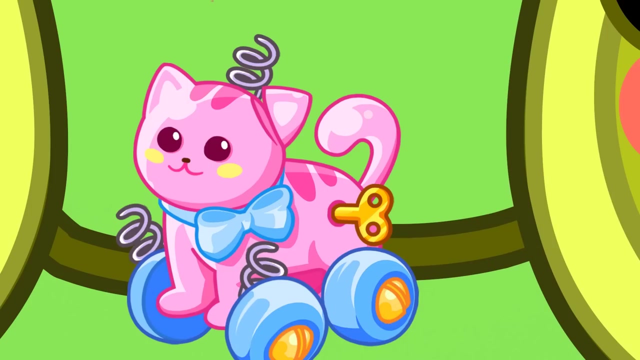 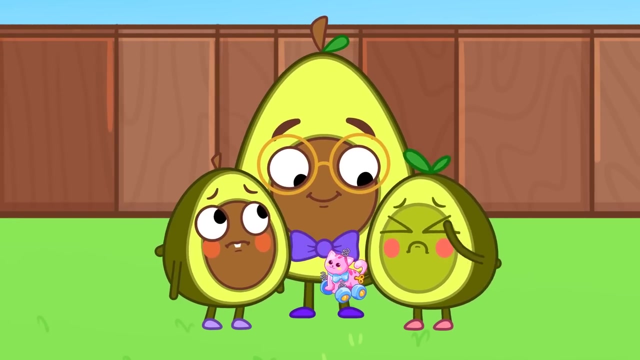 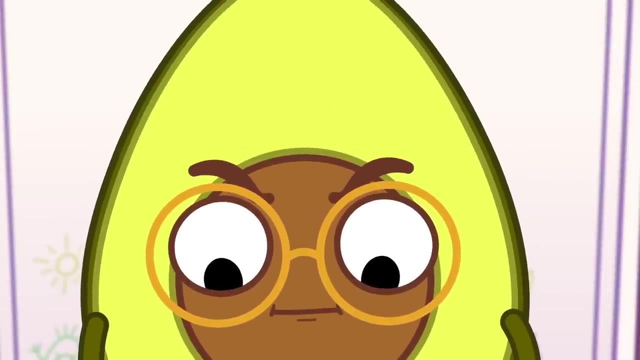 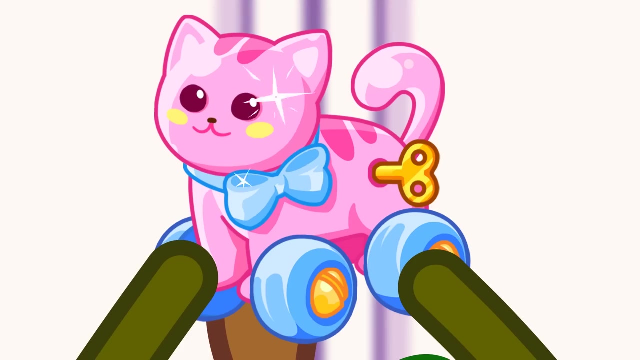 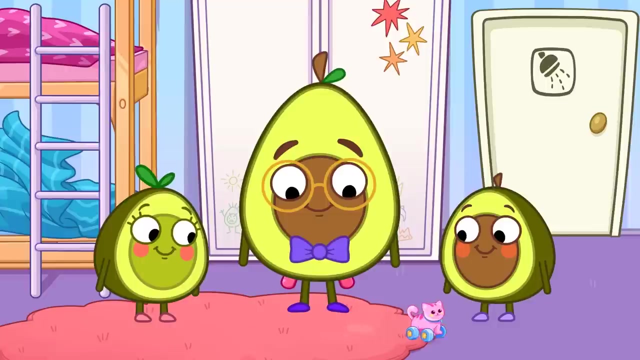 Why not ask Daddy for help? Pete, if you broke Penny's toy, you need to tell her about it. Penny is still looking for her missing toy. Daddy, can you help? I think I can fix it. Daddy did it. Thank you, Daddy. 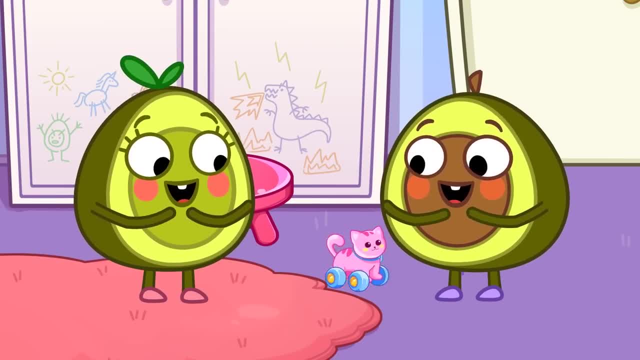 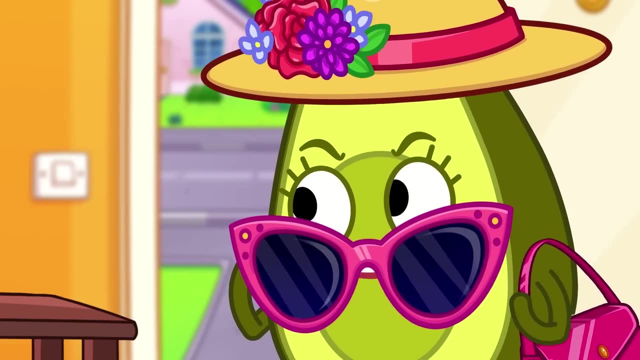 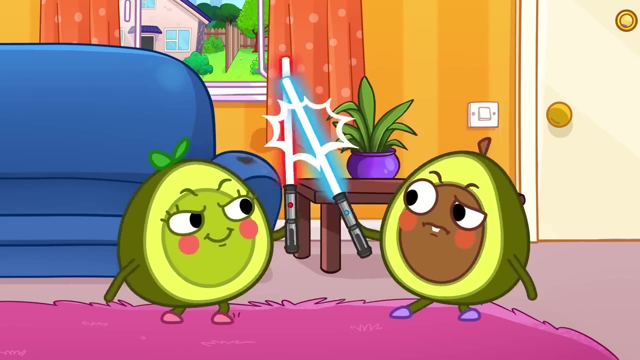 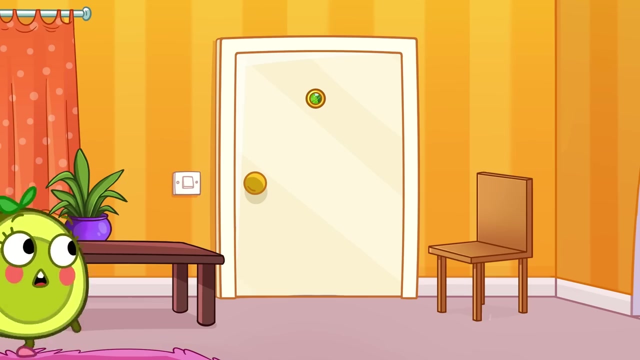 Be gentle, Pete. Bye. kids Play nicely and don't open the door to strangers. Pete and Penny promise to behave. There's someone at the door. Look through the peephole and see who it is. Open up. I have candy. 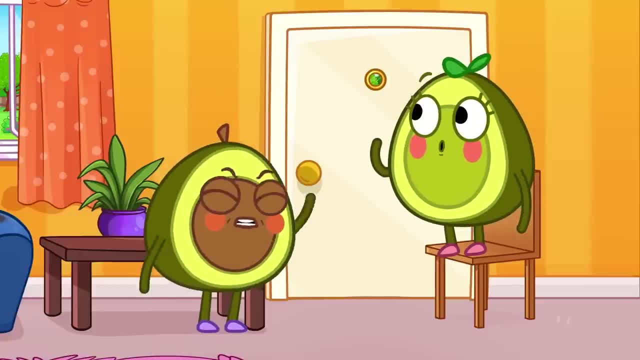 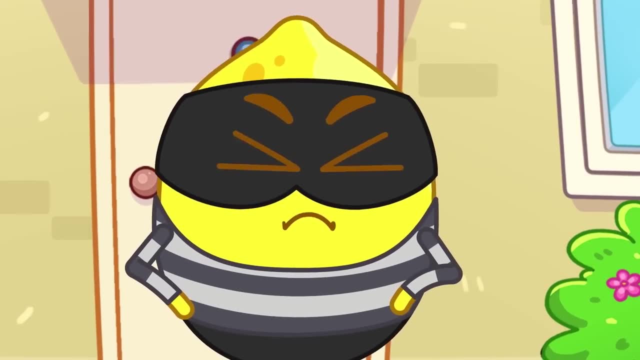 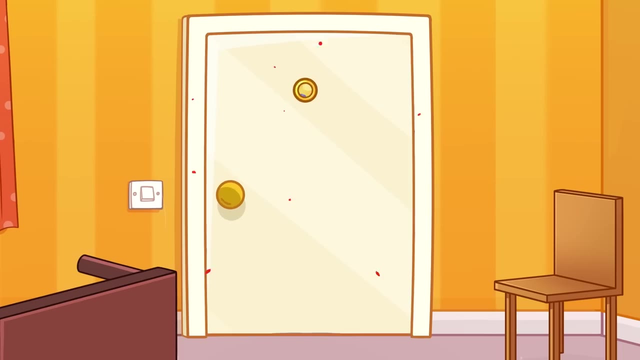 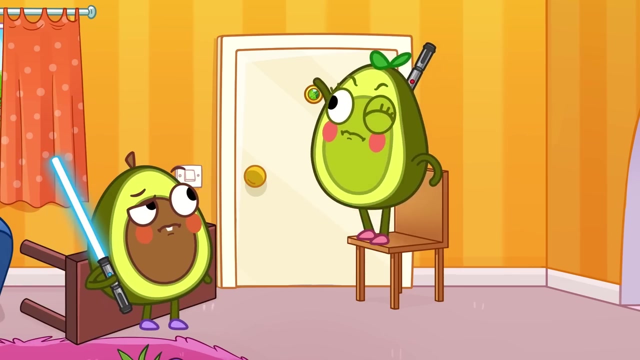 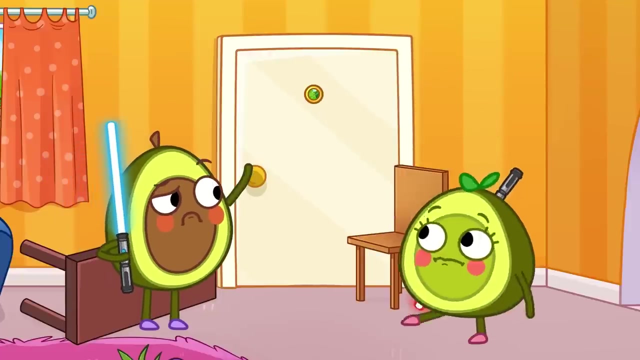 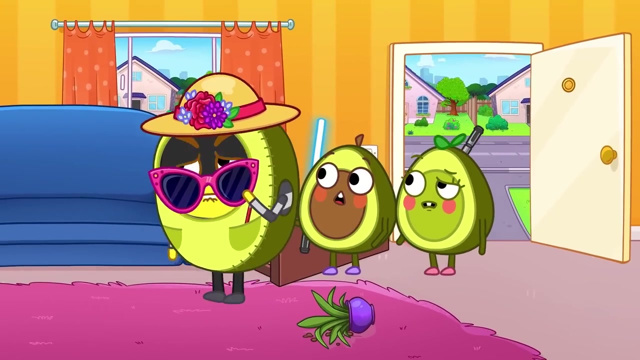 Should Penny open the door? We don't open the door to strangers. Mr Lemon has a sneaky plan. Now who is at the door? Open up. It's your mom. Mommy seems different. It's really Mr Lemon dressed as Mommy. 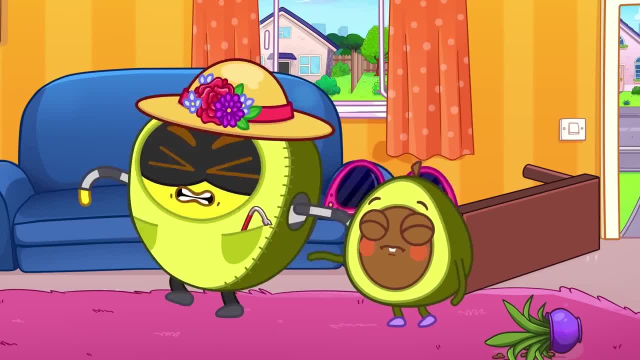 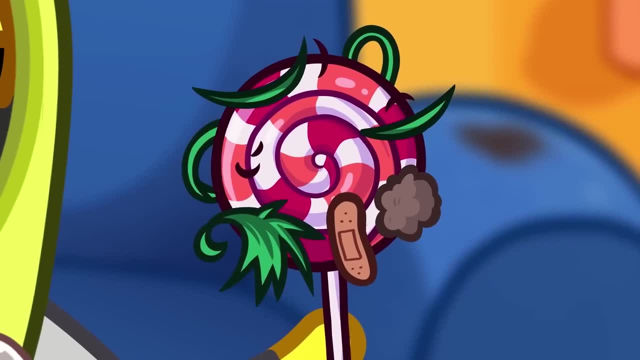 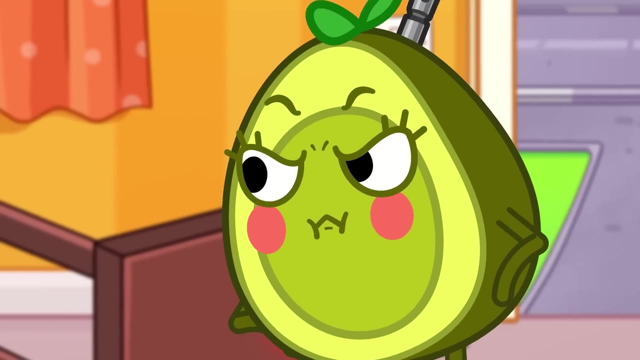 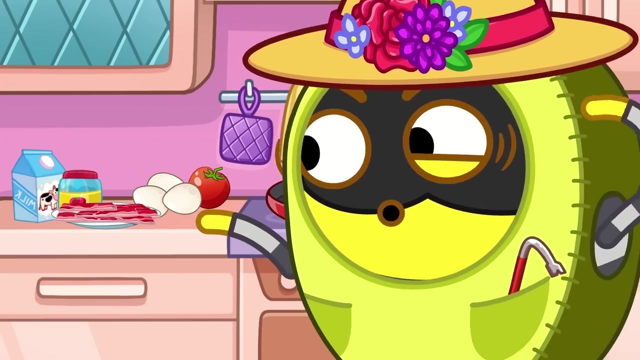 And he's up to no good. I'm hungry, Hehehe. Ew. That lollipop is covered in garbage. Penny is suspicious. this isn't Mommy's. Okay, I'll cook something. That's not how you make an omelette. 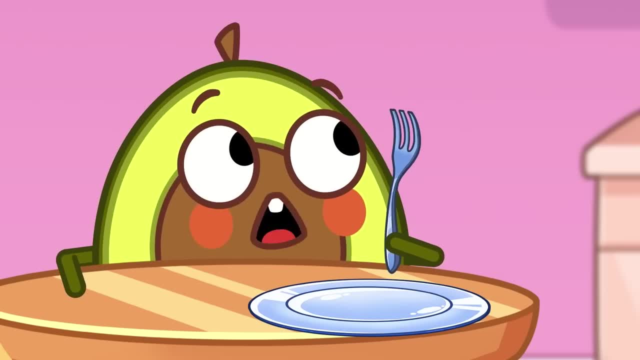 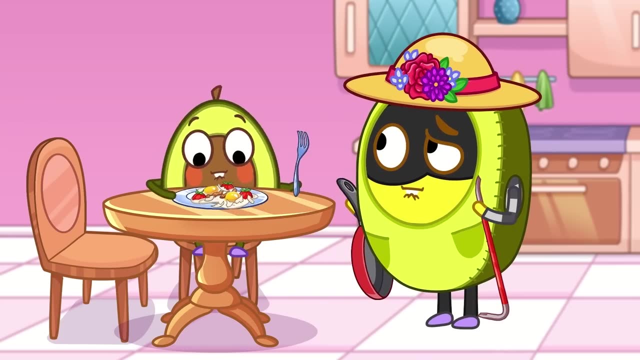 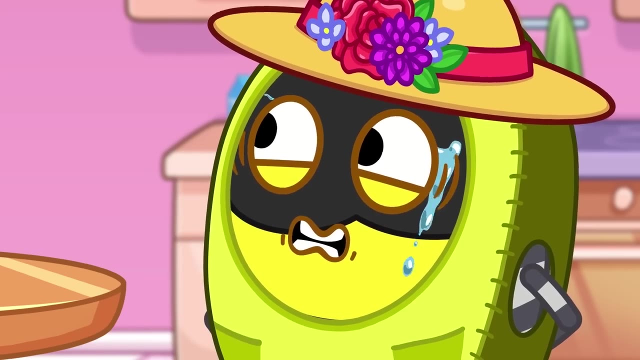 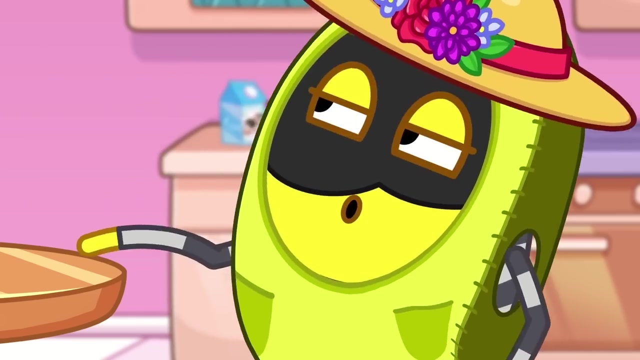 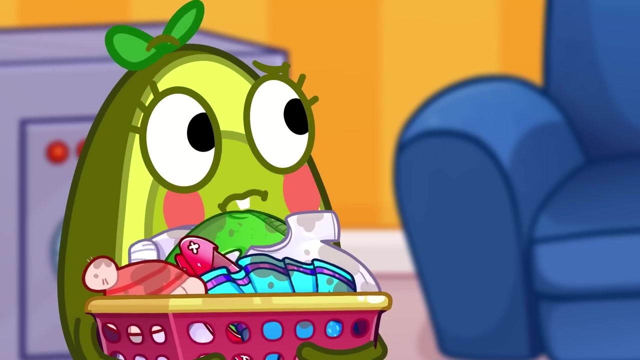 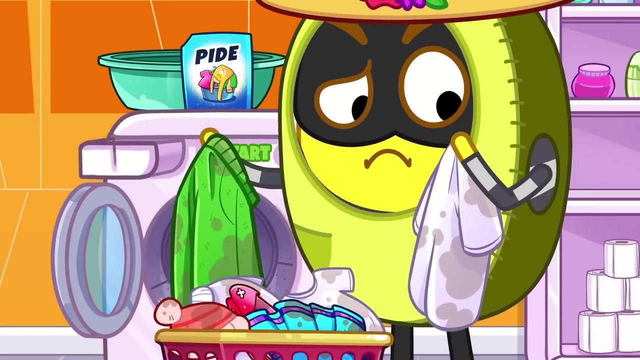 And it's stuck to the pan. Mom, Why don't you try your tire iron? Uh-oh Hee, hee. Do you like it? Pit, He does like it. You promised to wash my clothes. Mr Lemon doesn't know how to wash clothes. 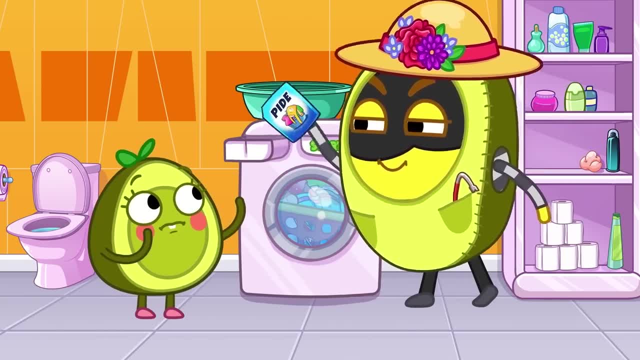 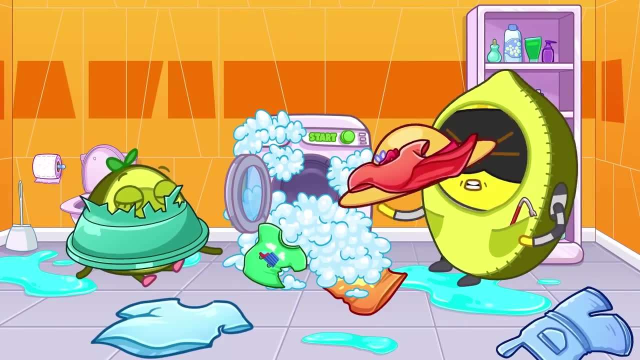 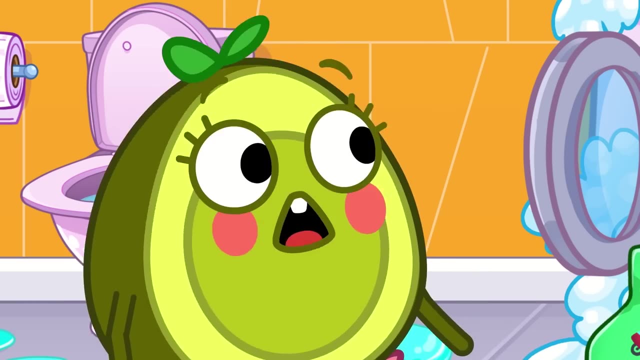 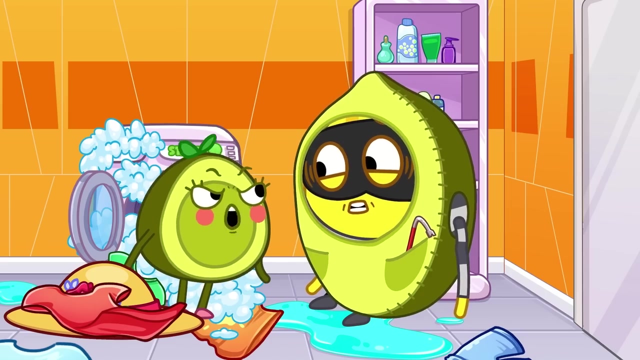 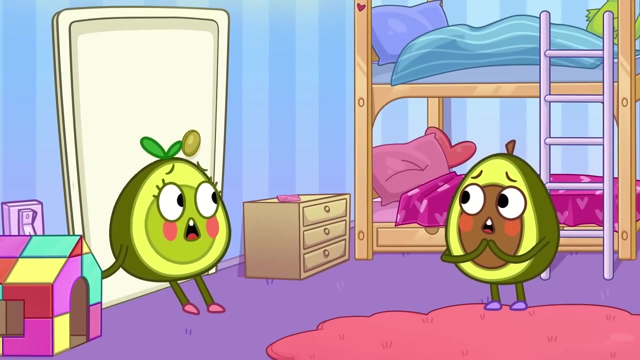 Mom, maybe it'd be better. Mr Lemon lost his hat And he knows this isn't Mommy. Mom, you're not our mom. I'm calling the police. Run, Penny, run. There is a stranger in our house. 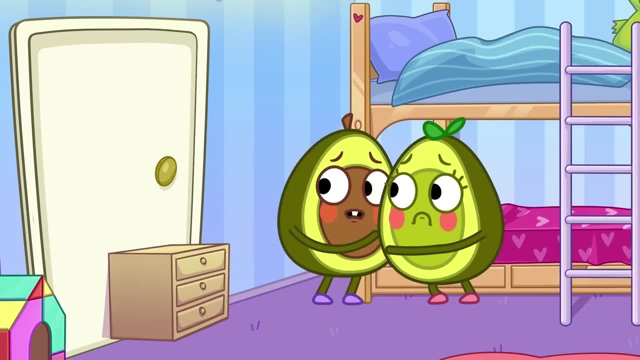 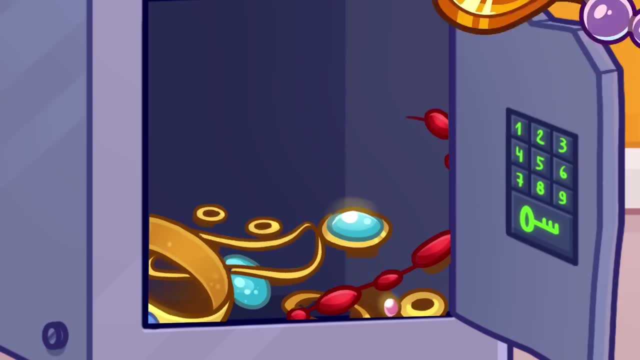 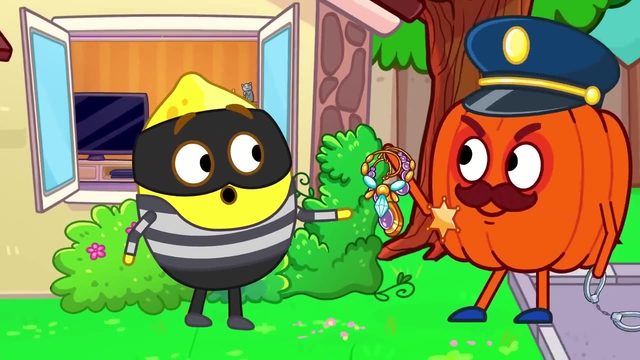 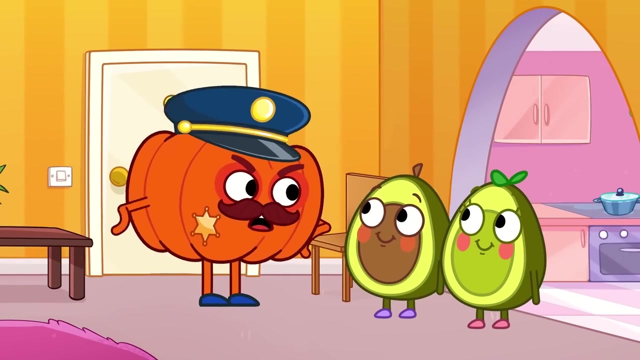 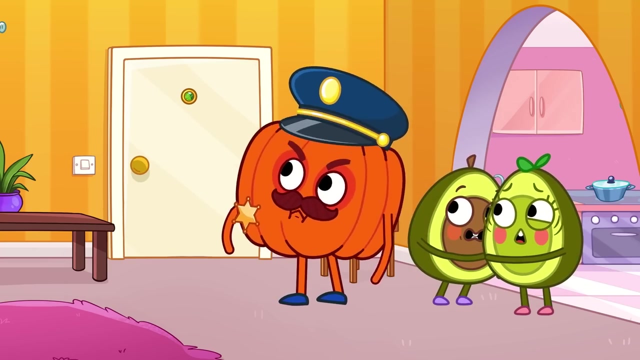 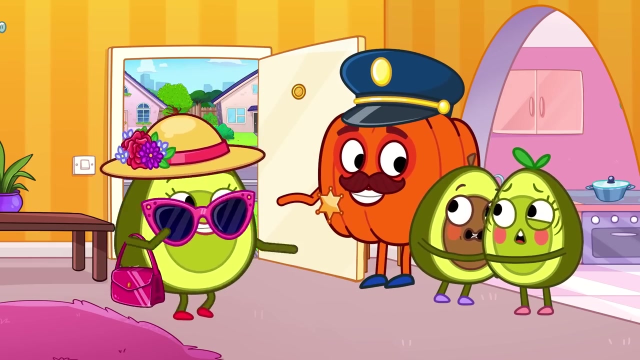 Help. Mr Lemon is breaking into the safe. It's full of expensive jewels. The police are here. Officer Pumpkin, arrest Mr Lemon. Do not open the door to strangers. Now who's knocking on the door? It's the real Mommy. 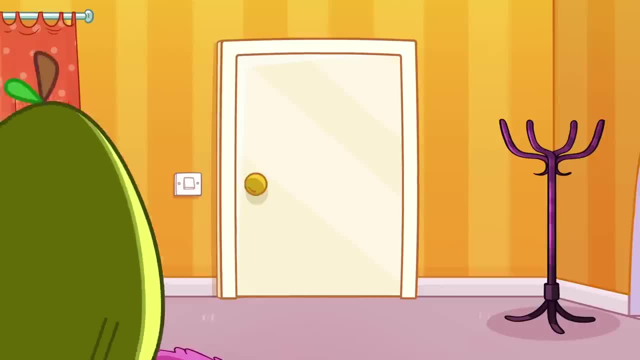 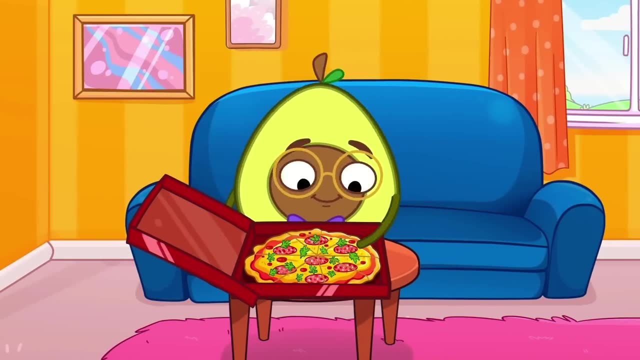 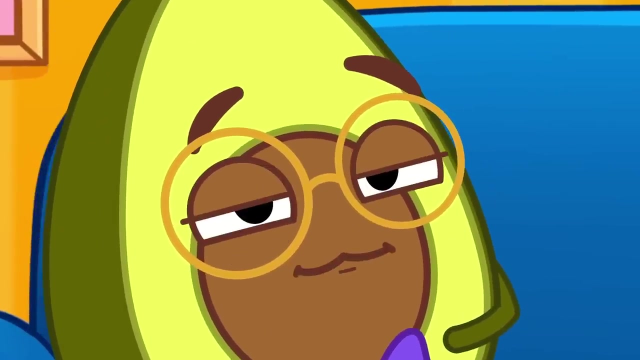 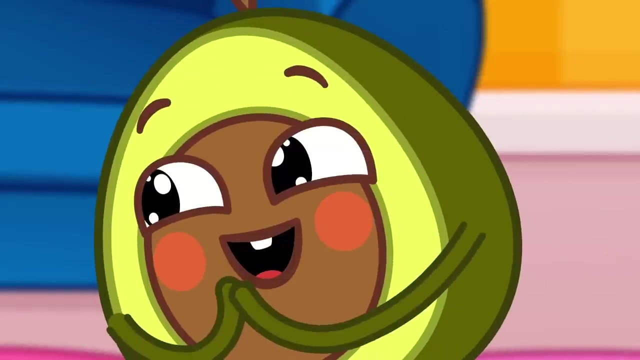 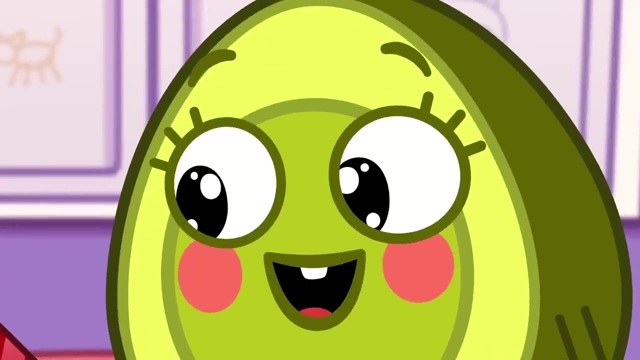 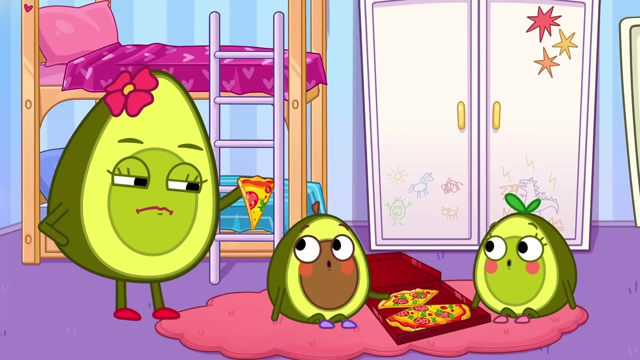 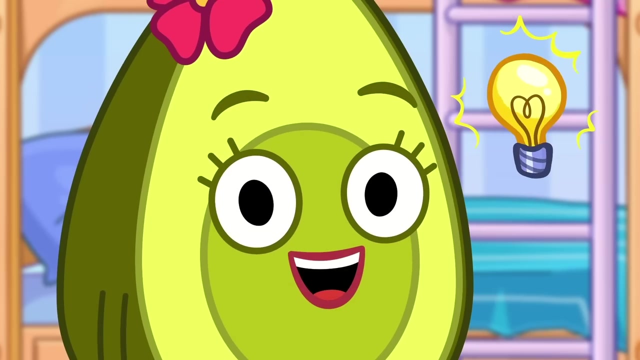 Hooray, Daddy ordered a pizza. Thank you, Mmm. Daddy's pizza looks so yummy, But Mommy thinks junk food is bad for you. Why not make a healthy snack? What does Mommy have in her bag? It's a. 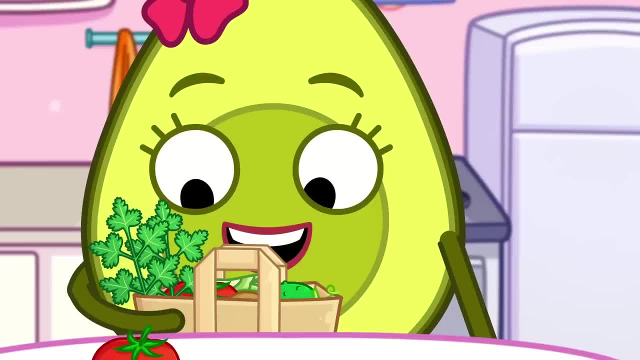 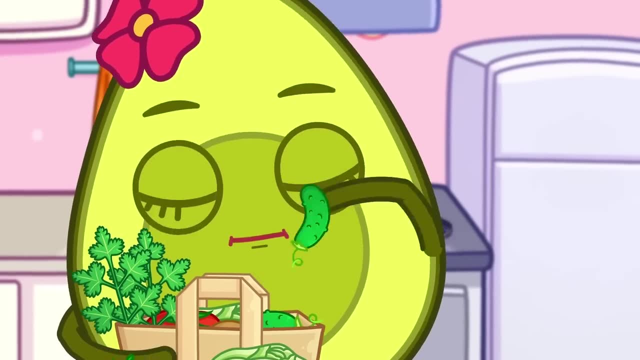 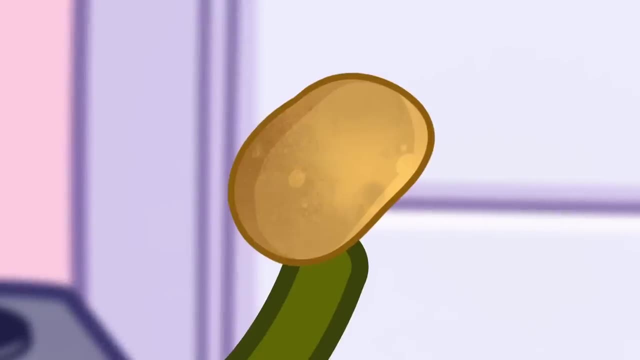 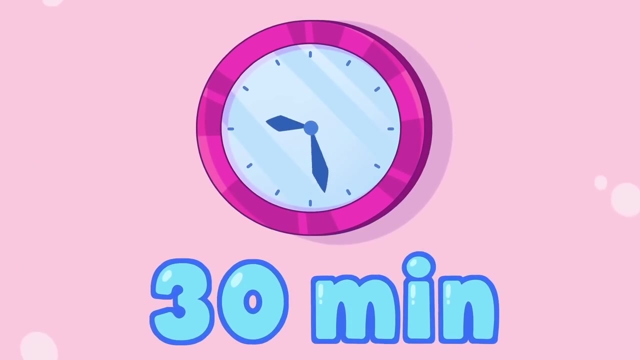 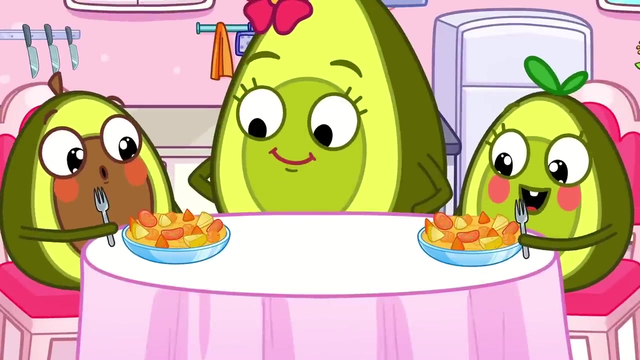 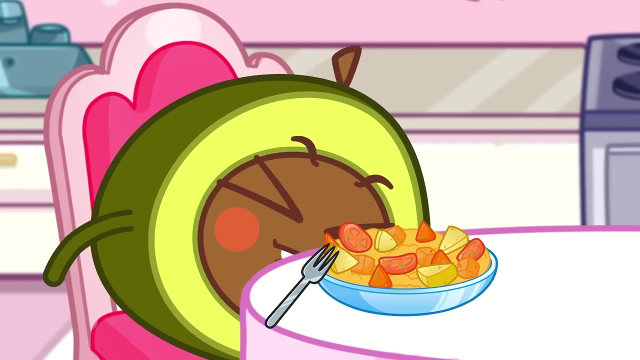 Tomato, And this Cabbage, And this is a Cucumber, And finally Potato. What will Mommy make with these? Mommy has made a healthy snack. Wow, Cola isn't very healthy. Ahem, Ahem. 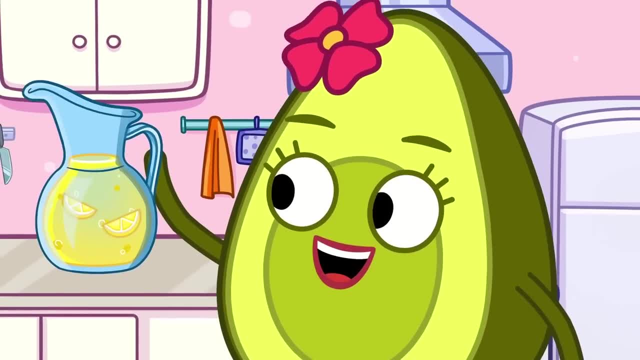 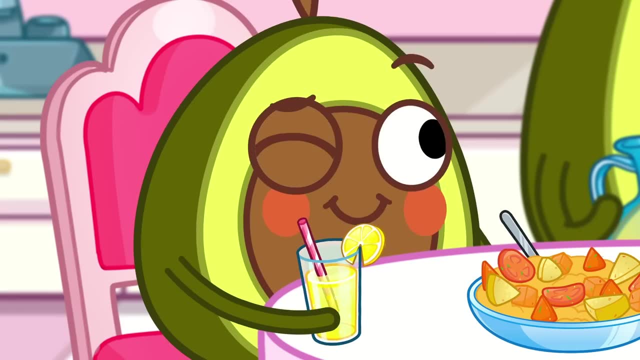 Uh oh, Tomatoes got in my eye. OK, Me, amblr FOW 3, I got an idea. Let's have a potato stand. Oh my sweet, no 班 depende. That's what I'm talking about. 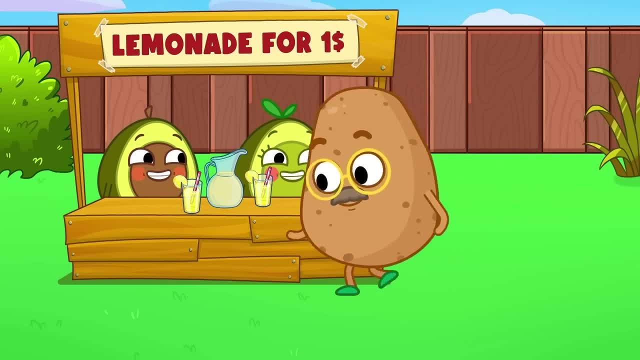 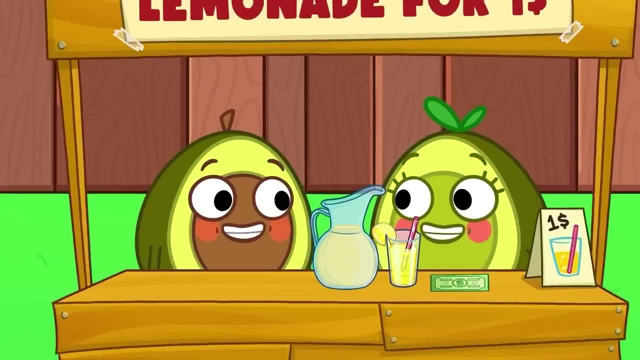 OK, Okay, Pay the staff. Tap, Tap, Tap Flies their feet outside the tap. Let's see who can eat one now. Oh my, Let's see if I seasons closing up, Aren't you real? No, I'm the Big Sean. 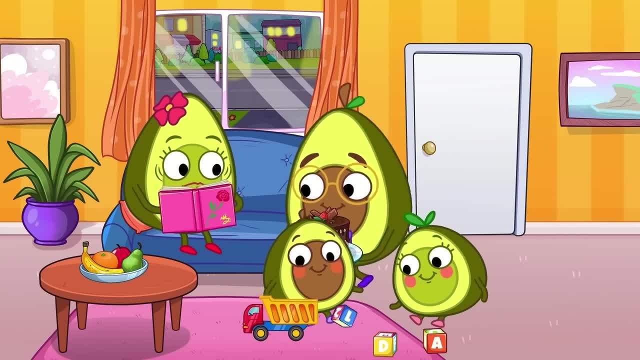 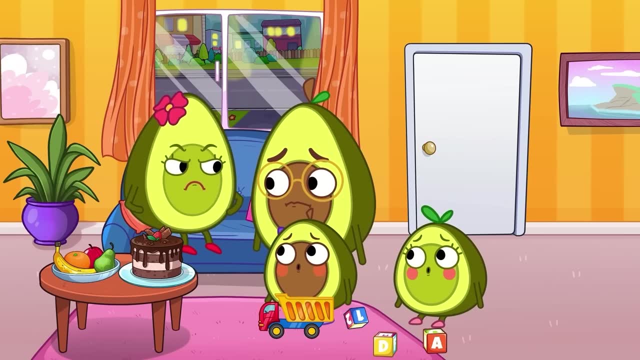 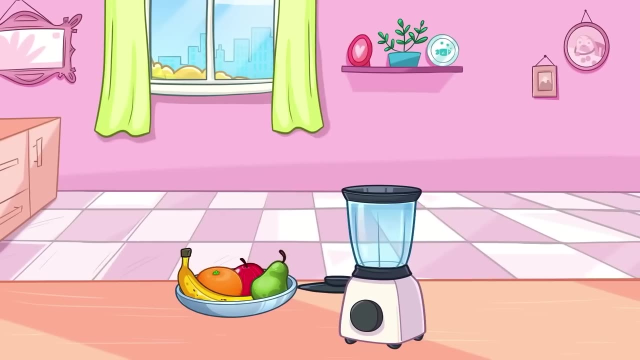 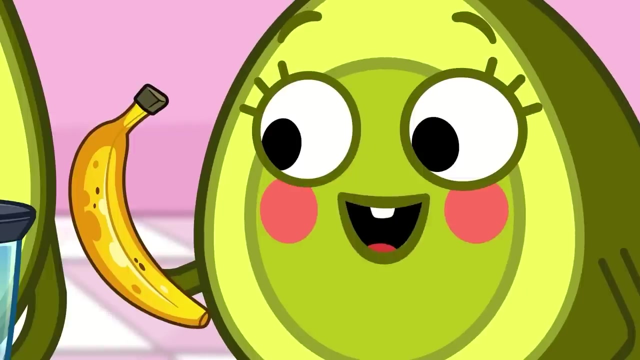 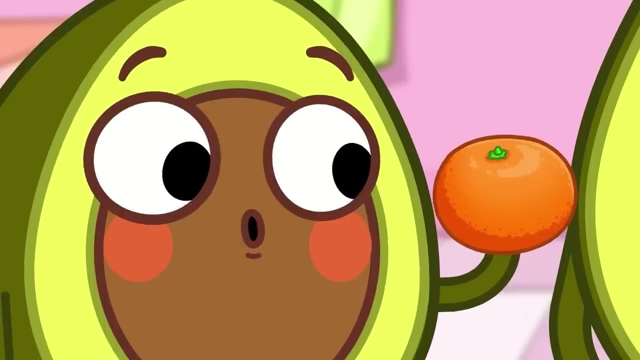 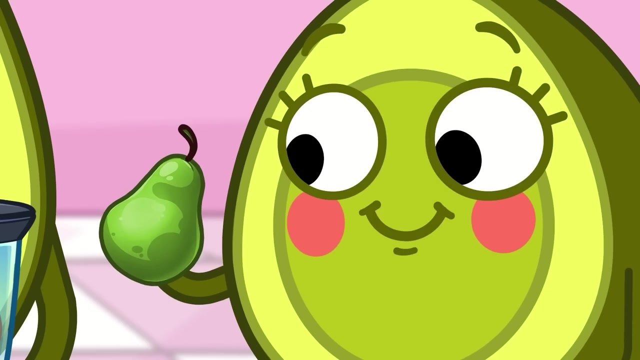 Daddy has brought home a cake. Mommy thinks fruit is a better choice. Let's make a smoothie. You need an… Apple And a… Banana. Anything else Orange, And one last thing: A… Pear. Now we blend it all together. 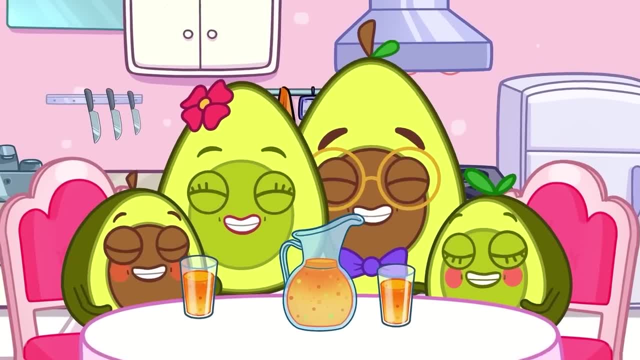 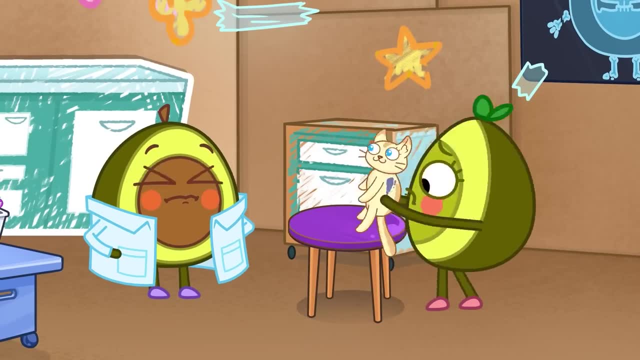 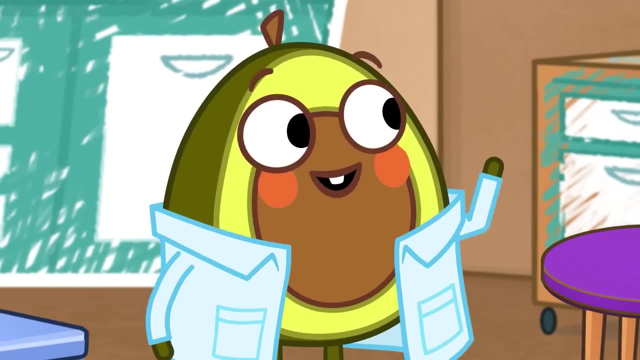 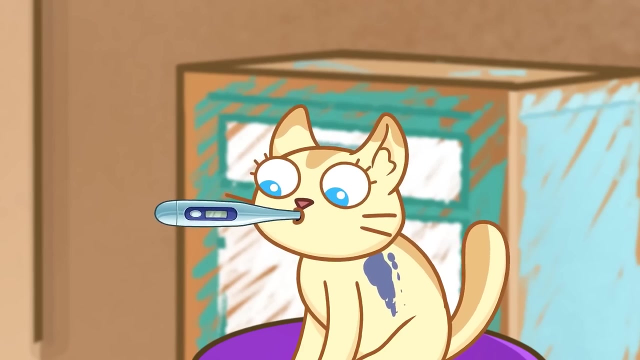 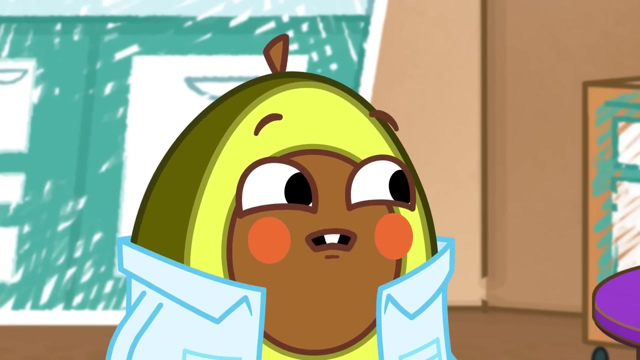 Healthy and delicious. Bye. What's the matter, Penny Doctor, Save the kitten. No, He has a bruise. Doctor Pitt should do some tests. Does Kitty have a fever? The temperature is normal. Check Kitty's heart with stethoscope. 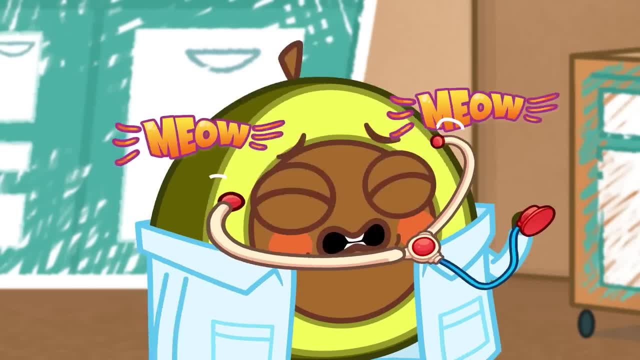 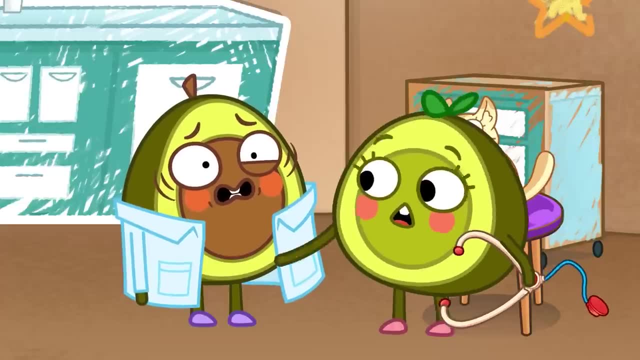 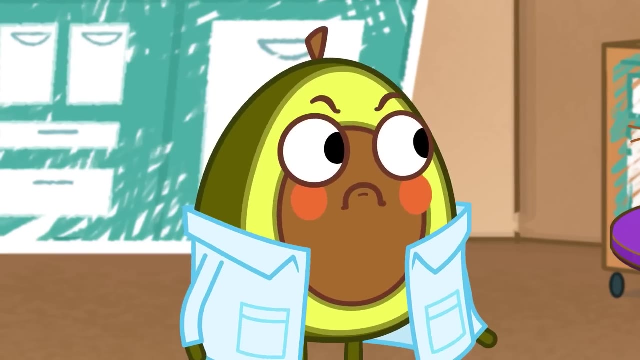 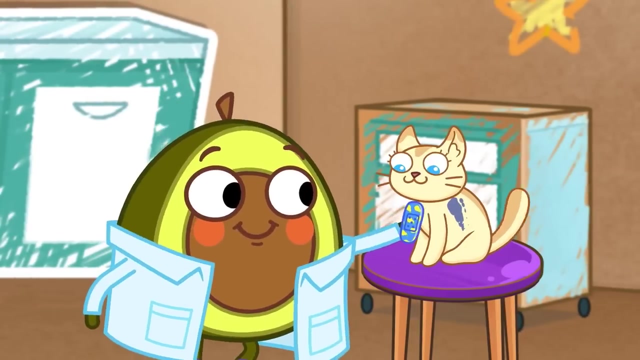 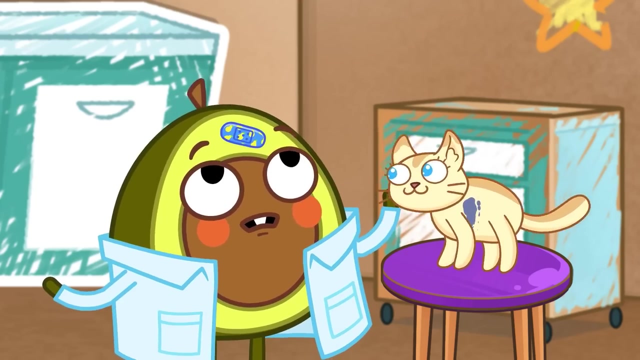 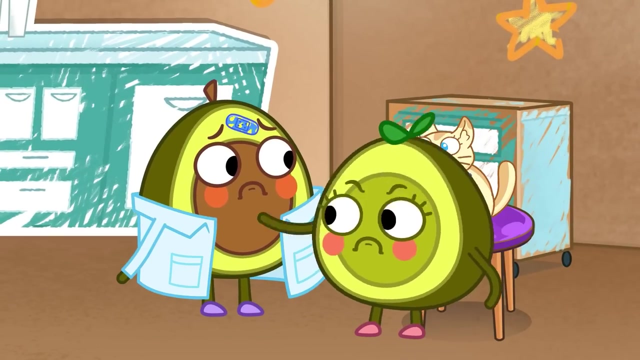 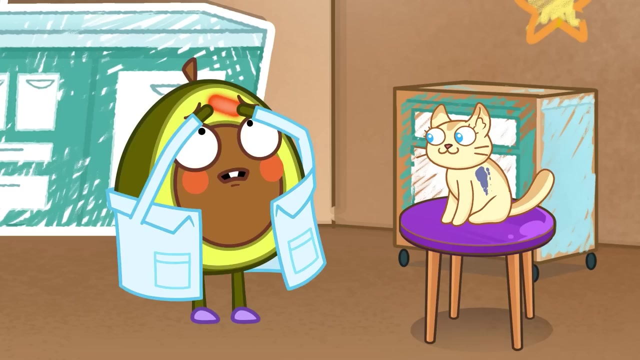 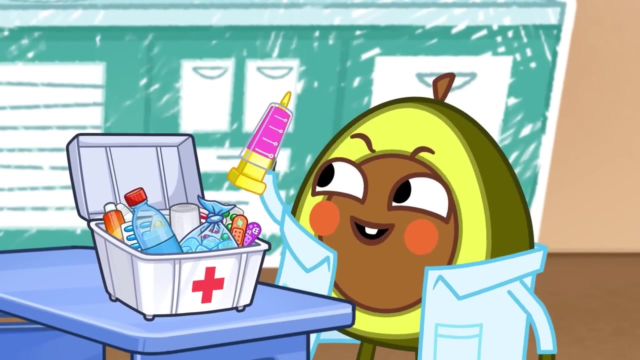 Meow, Can you help Pitt Penny? Maybe a bandage will help. Kitty wants to play. And now the bandage is on Pitt's head. The examination is over. It's time for treatment- Time to give Kitty a needle. 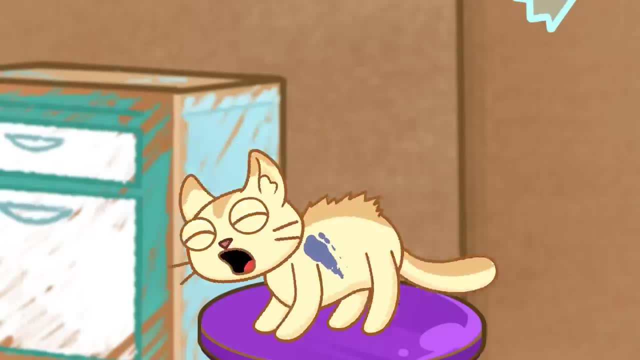 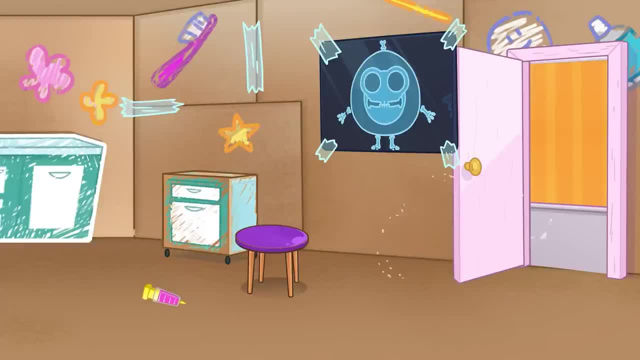 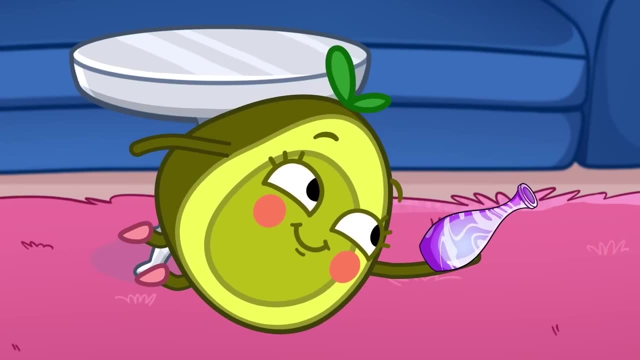 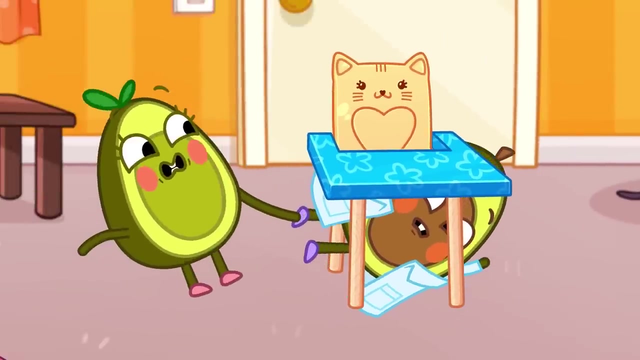 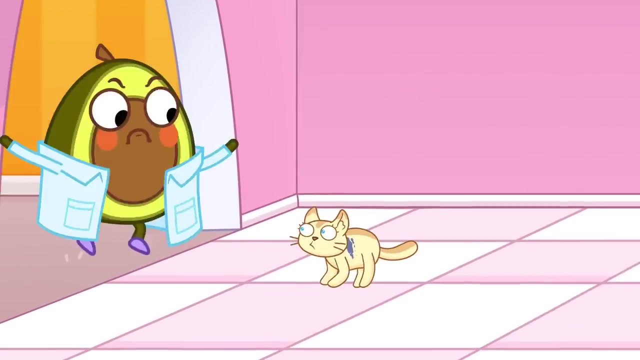 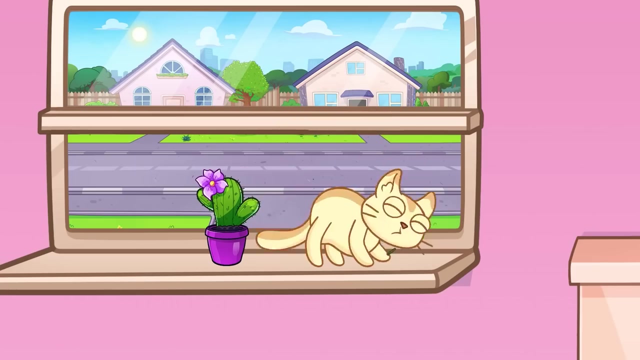 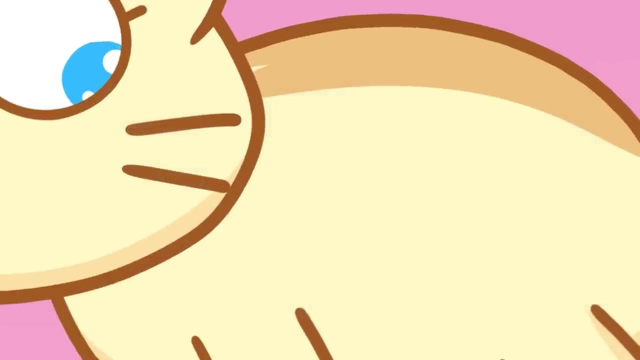 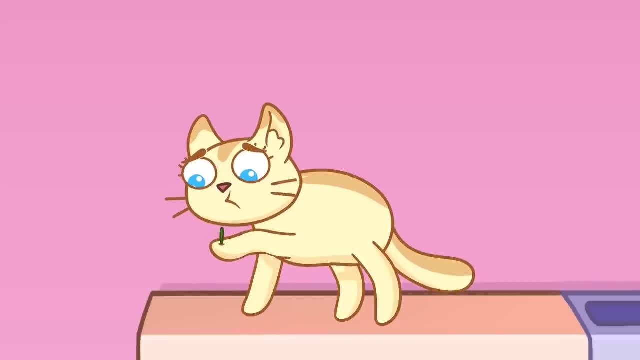 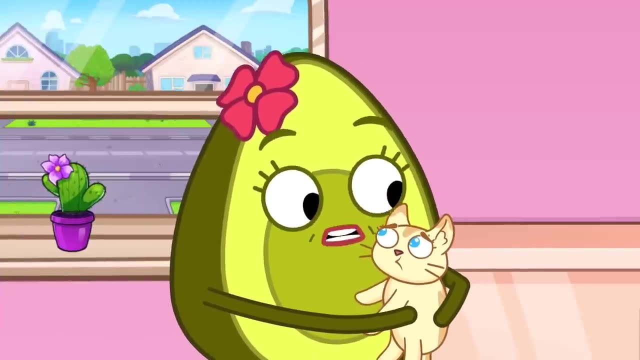 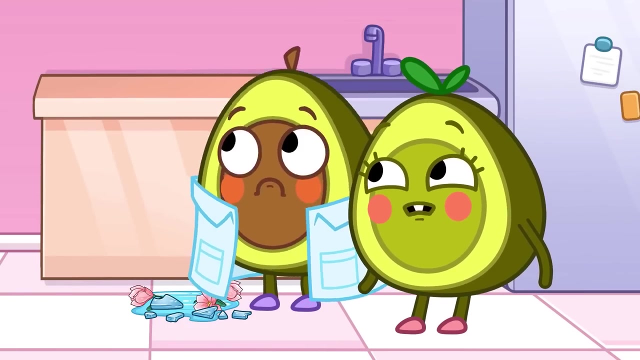 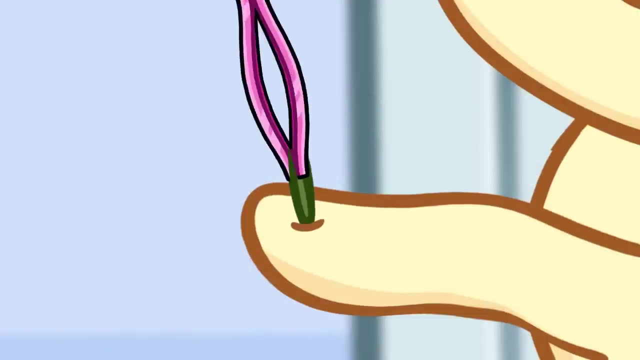 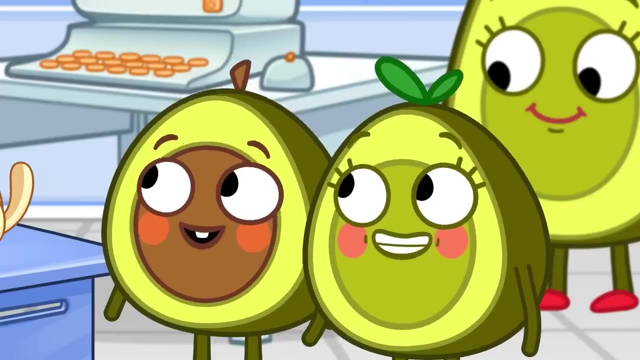 He's not sick, But there's something in her paw. We need to take him to the wet. Who is that? A vet is a doctor for animals. Kitty's paw is fixed. If your pet is sick, the veterinarian will help. Thank you for helping Kitty, Mr Vet. 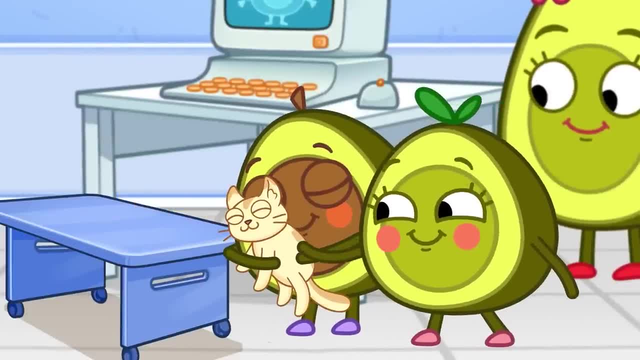 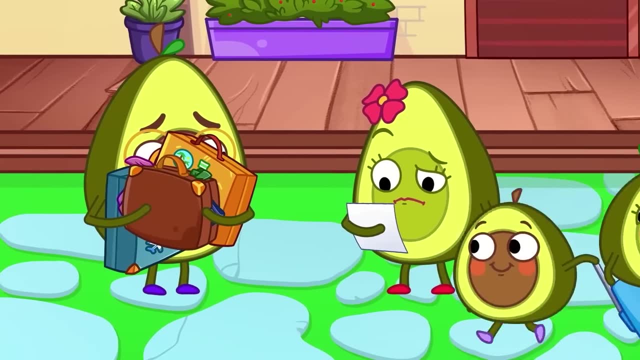 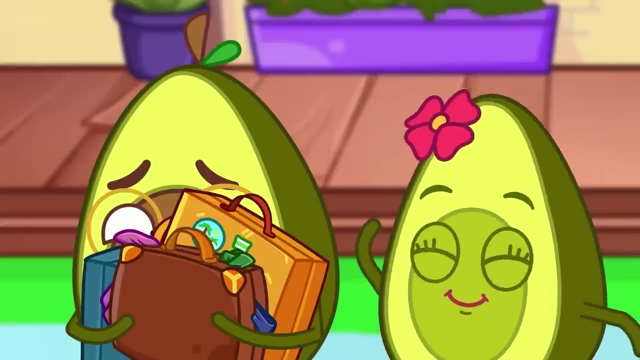 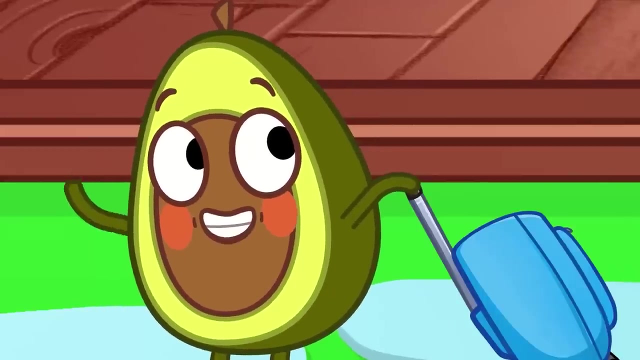 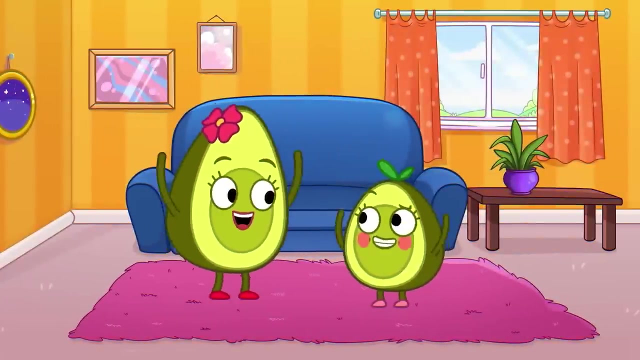 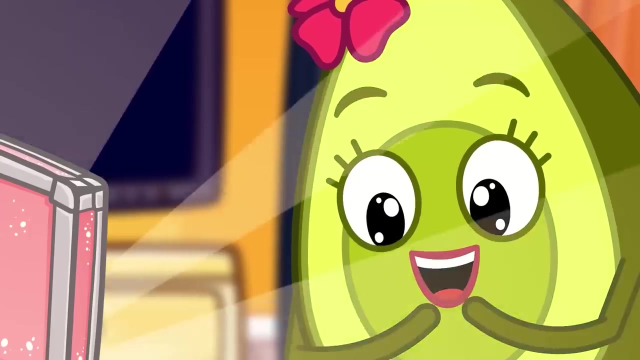 Daddy's bags are packed And Pit has his suitcase. Now Dad and Pit are ready for their trip. Have fun, Pit and Daddy. Penny and Mommy are excited. Penny, let's spend the day together. Penny has an idea What's in the case: It's a makeup kit. 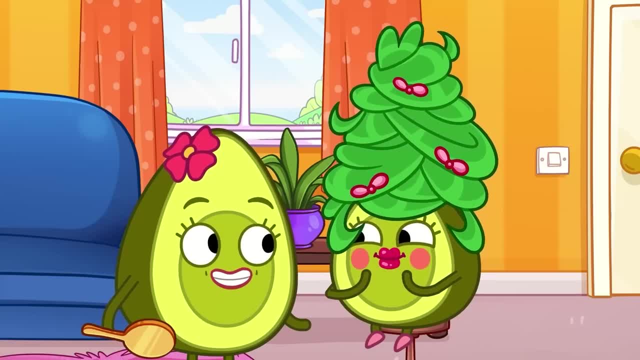 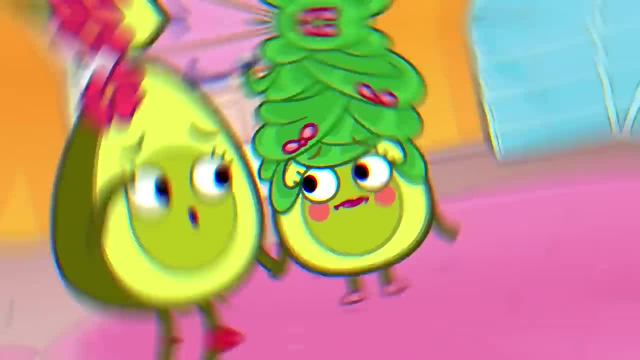 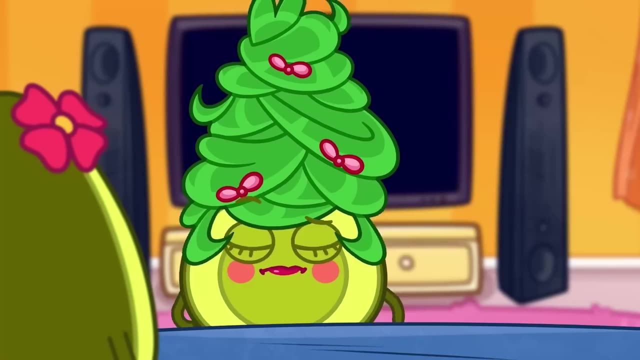 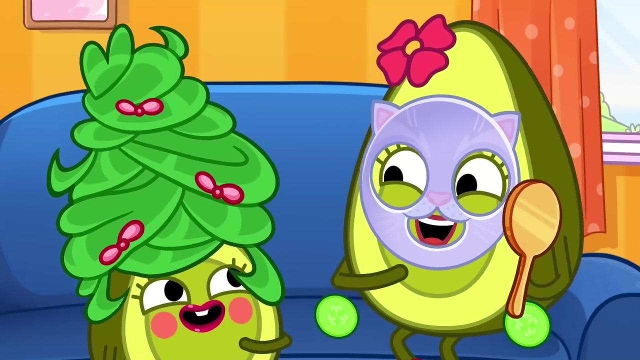 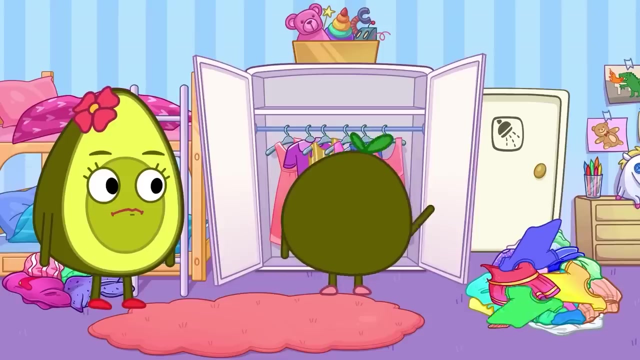 Now Penny looks like a supermodel. Penny, pretend you're on the runway. Thanks, Mommy. Have a seat, Mommy. This mask will help Mommy relax. See Mommy, Now for a game of dress-up. Oh, Maybe Penny's a doctor. 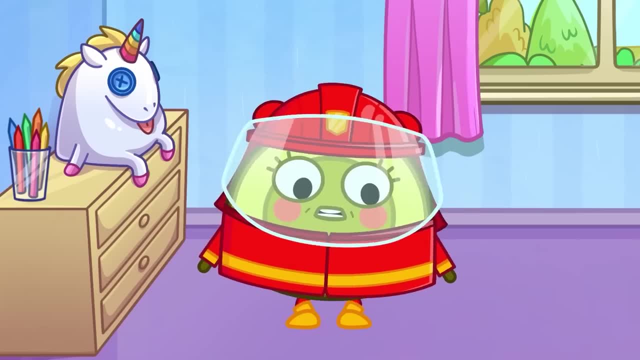 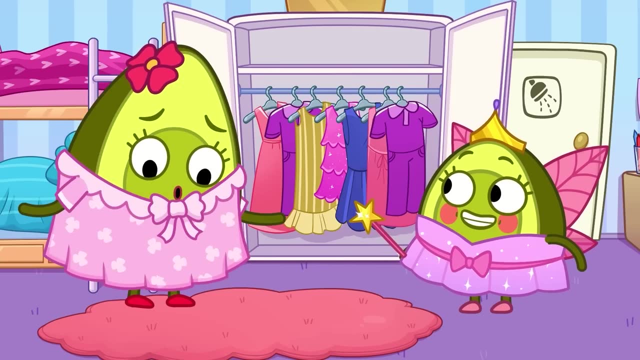 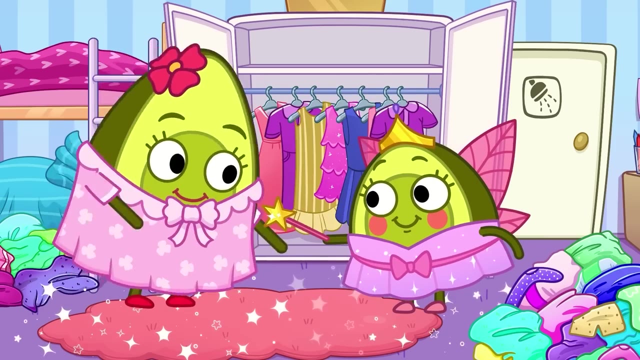 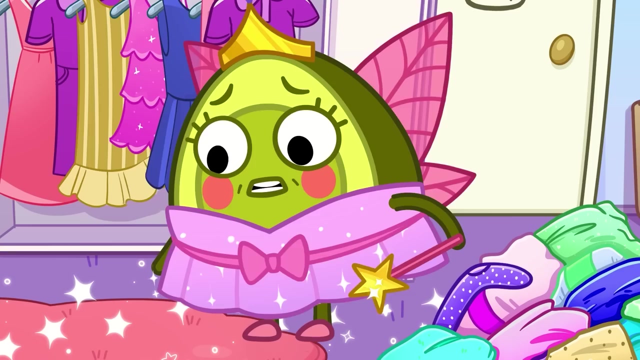 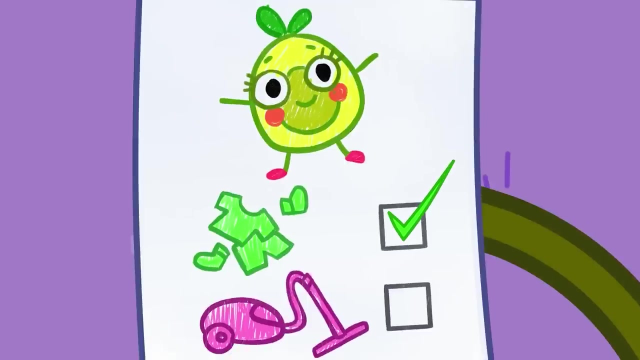 Penny's a duck, Penny's a fireman, And now she's a fairy. Mommy needs a dress too. What a magical dress. What's wrong? So we need to clean the room. Penny doesn't want to, She doesn't want to. You need to clean and vacuum. 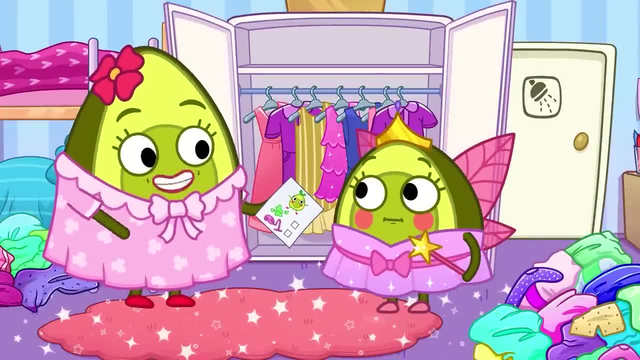 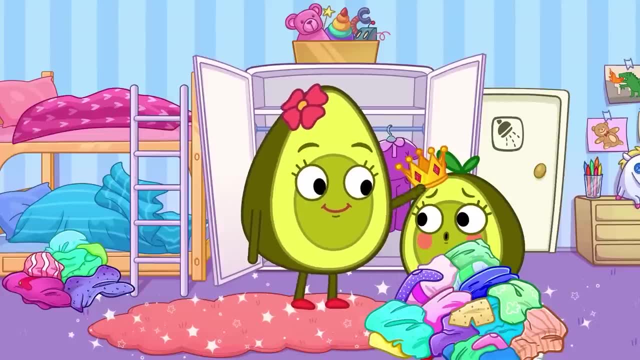 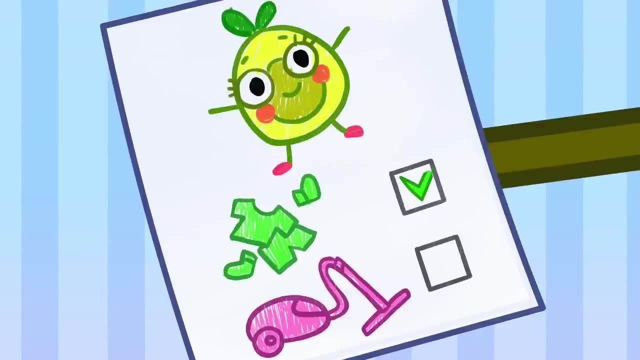 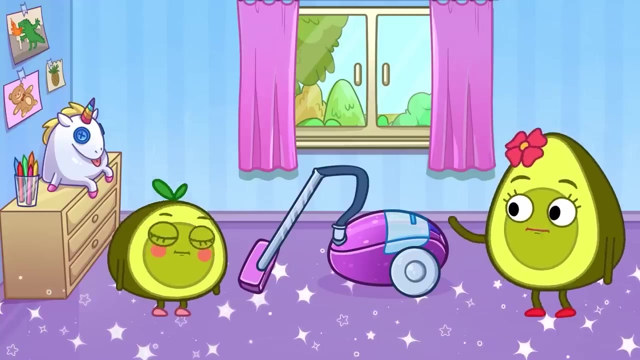 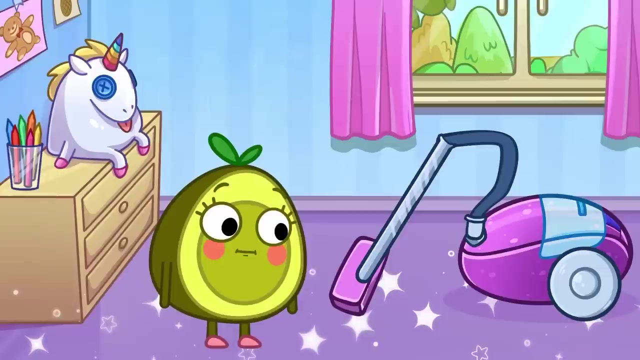 Penny, please help me clean up and fill in the circles. All the clothes must go back in the closet. All done, Check. Now it's time to vacuum. I'll be right back. Don't turn on the vacuum cleaner yet, Penny. you should wait for mommy. 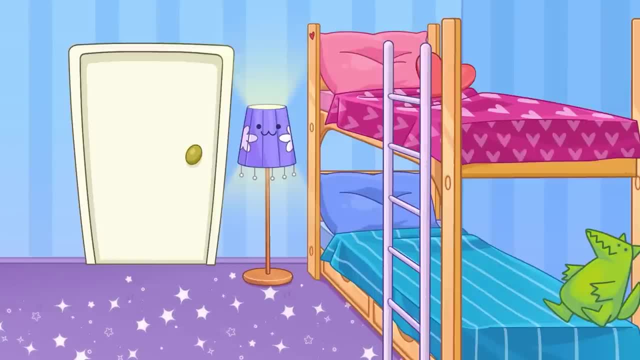 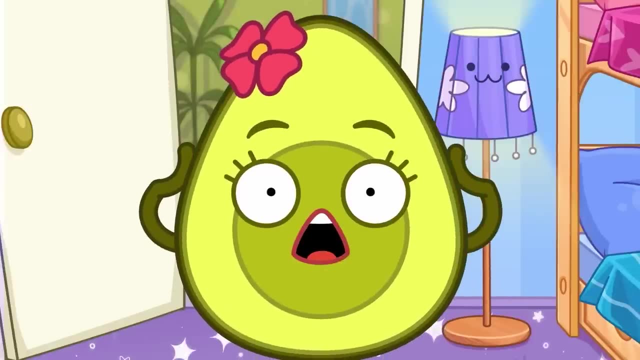 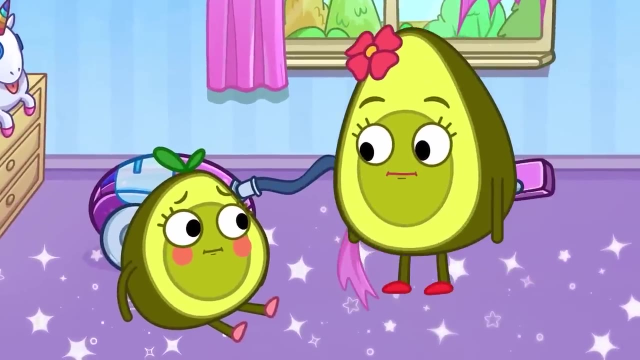 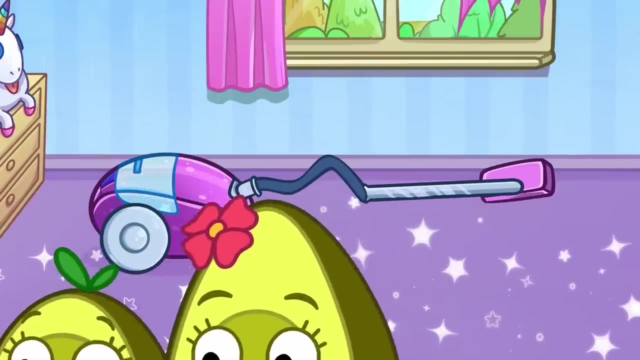 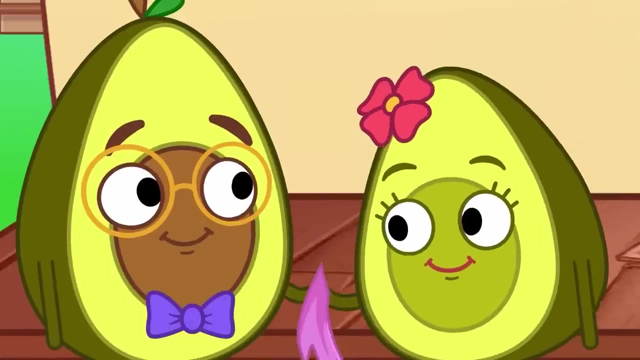 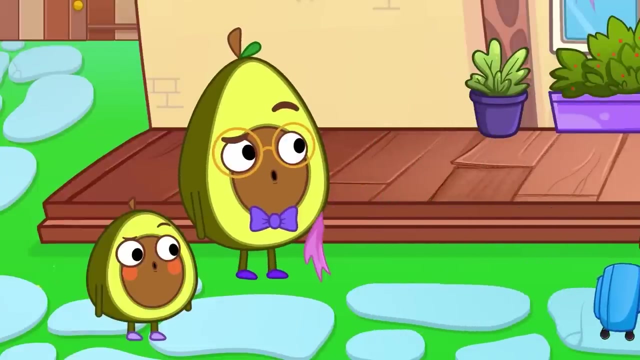 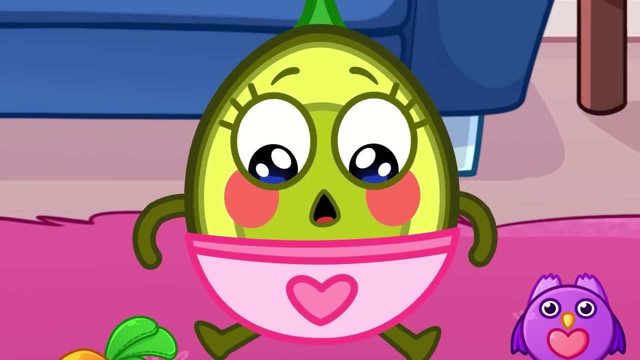 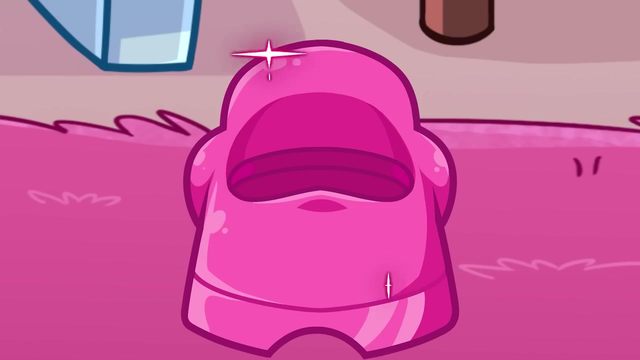 Oh no, Penny needs help Now. the curtains are ruined. Penny, never use the vacuum cleaner without me. Who's at the door? It's Pit and Daddy. Welcome home. Poor baby. Penny wants baby to use the pink potty. 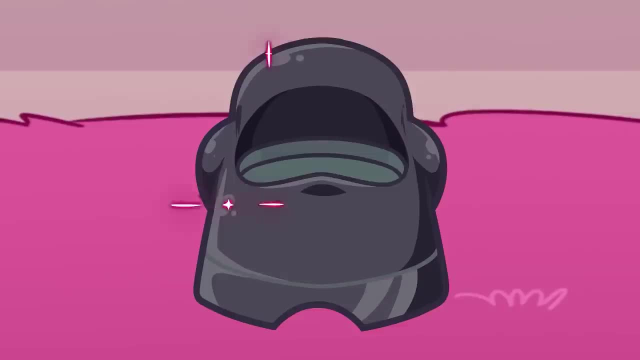 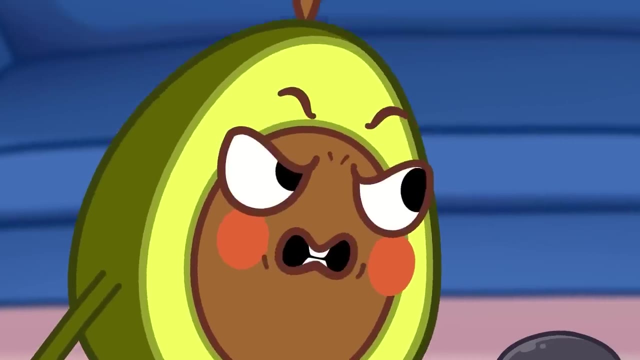 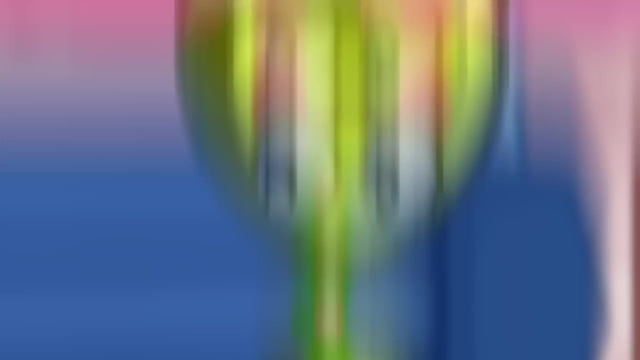 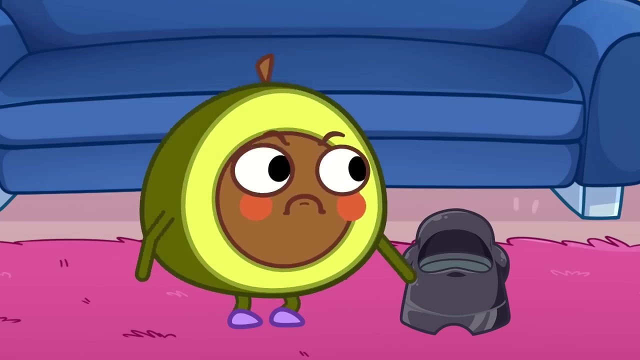 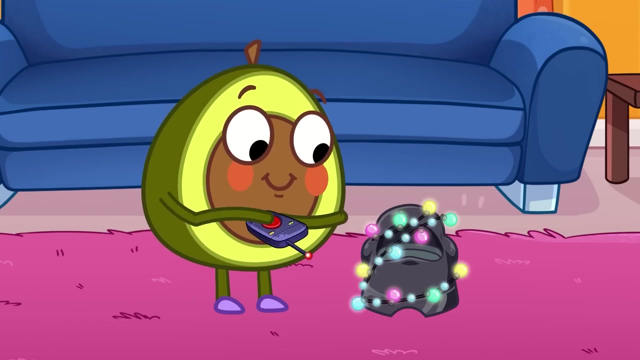 Pit wants baby to use the black one. Pete Pink is better. But Pit doesn't agree. Black is better than pink. Which potty will baby choose? Pit has an idea. He'll add pretty lights. Hey, look at this. 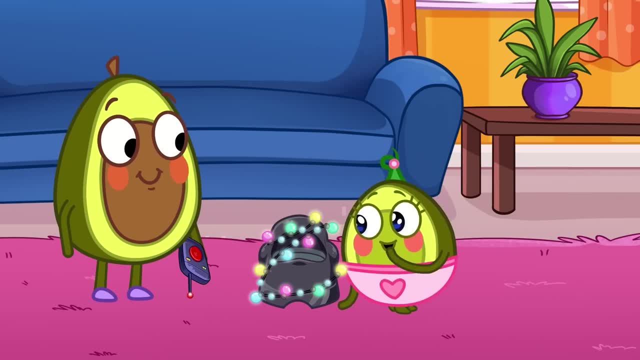 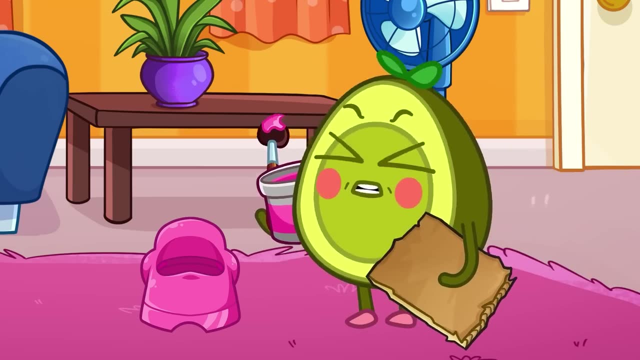 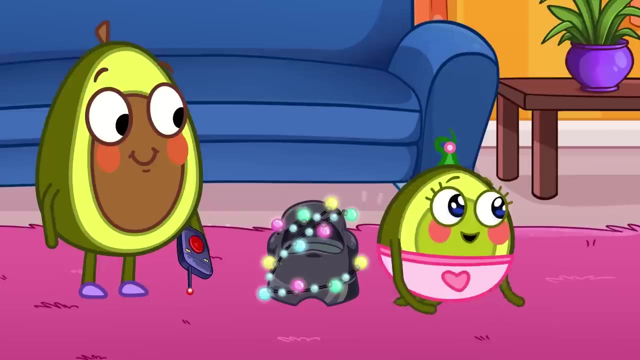 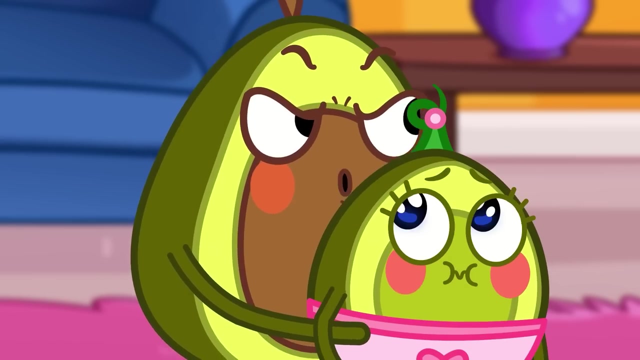 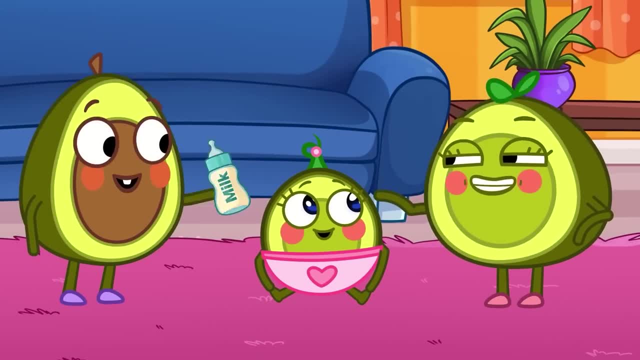 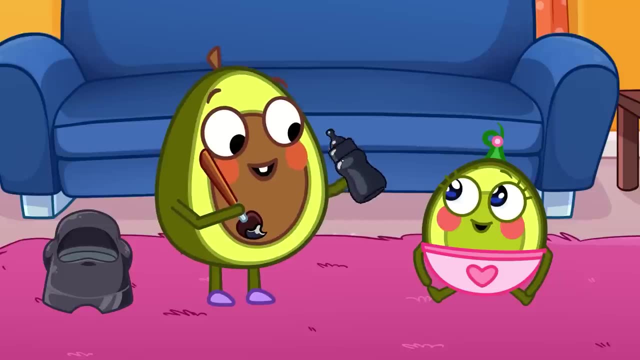 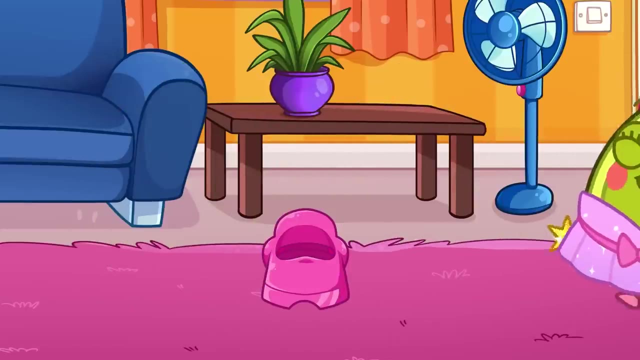 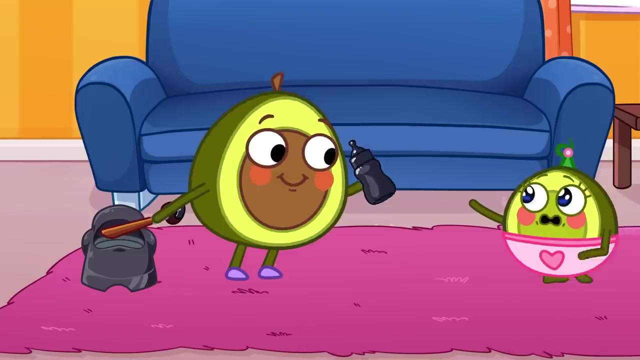 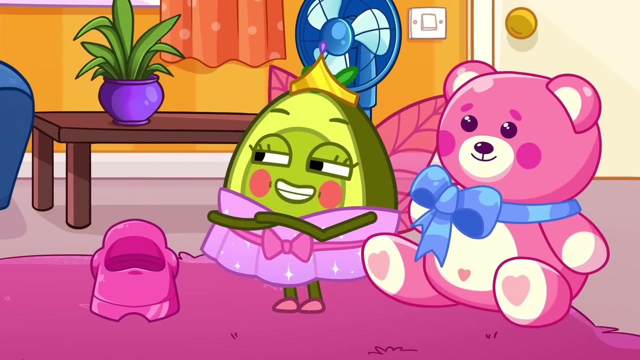 Poor Pit. Does Baby want milk? She'll need to use the black potty to get some. Now, Penny is a fairy princess. Sorry, Penny, but Baby's hungry. A pink teddy bear might attract her. A pink teddy bear might attract her. 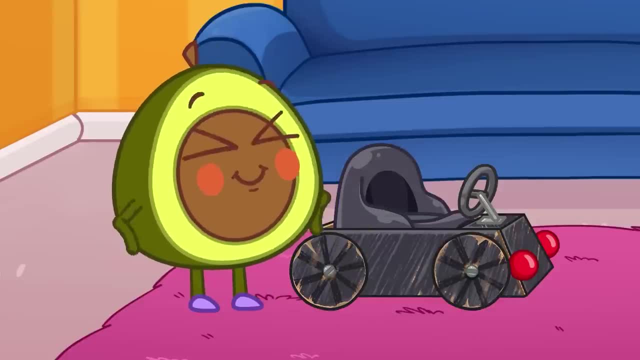 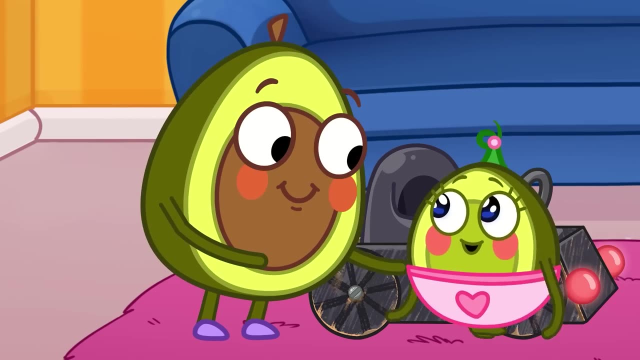 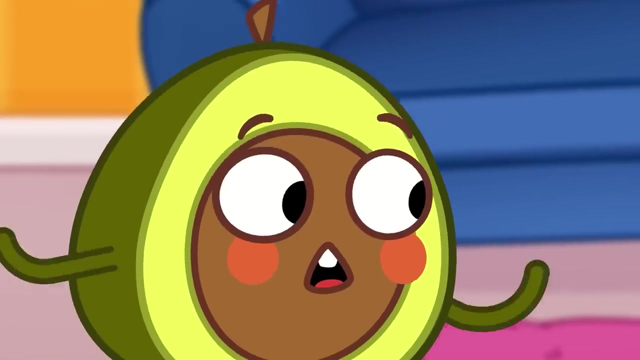 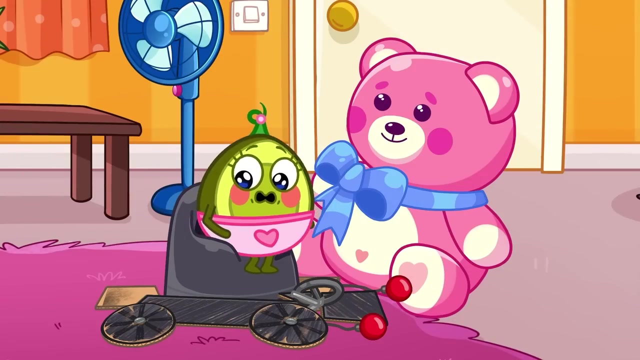 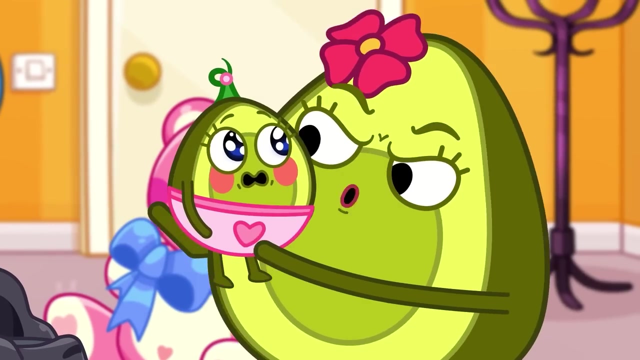 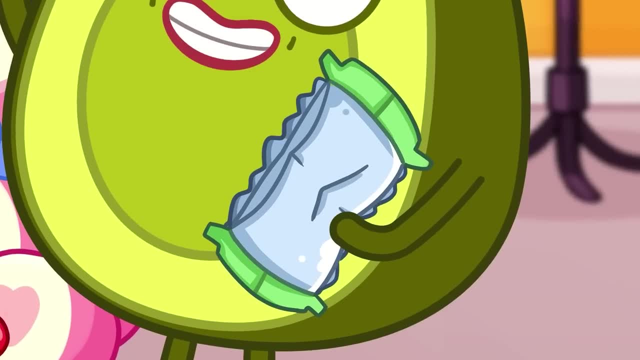 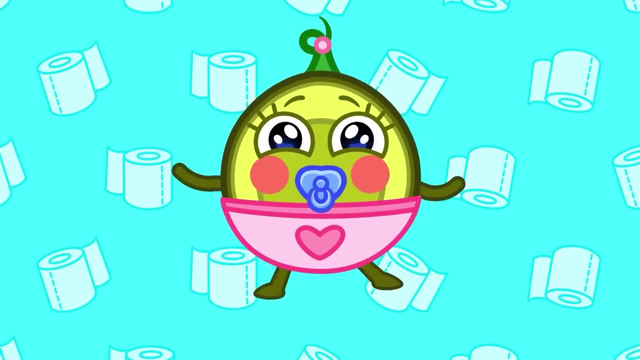 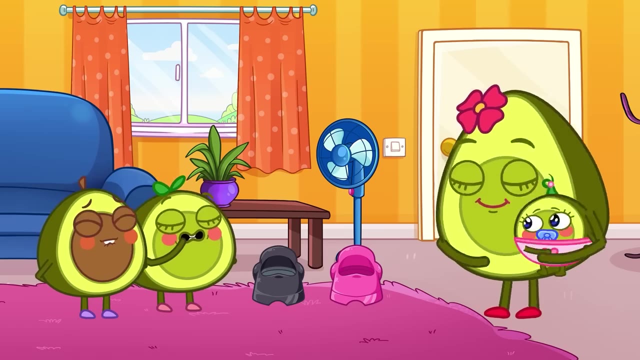 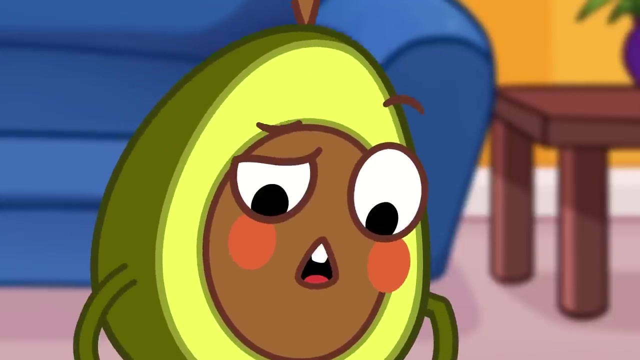 She just need a diaper change. Let's get rid of the old diaper And give her a new one. It's too early for her to use the potty. That's why babies wear diapers. Now. Pit needs the washroom. Hurry Pit. 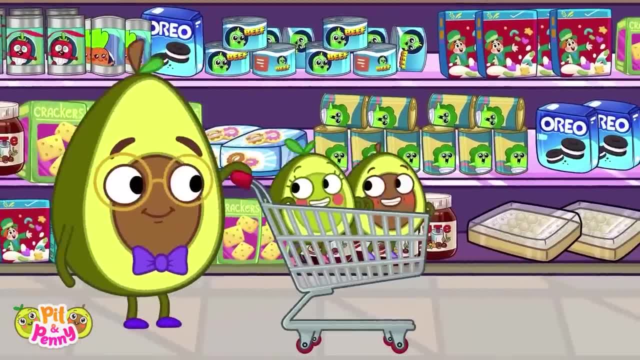 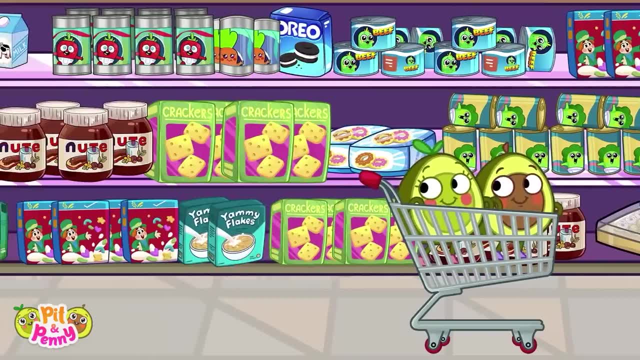 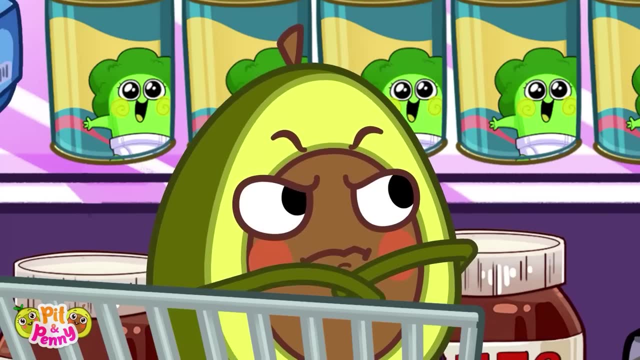 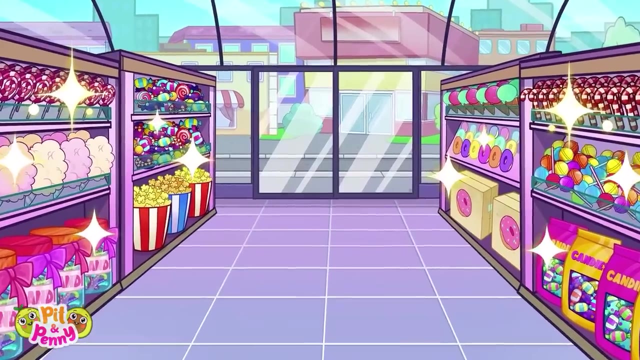 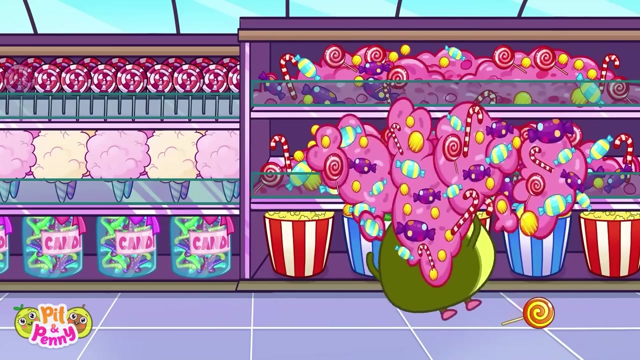 Pit and Penny are shopping with Daddy. I'll be right back. Please don't wander away, Penny. you should stay in the cart. Looks like Penny found the candy aisle Careful. Oh, it's Mr Lemon. What is he up to? 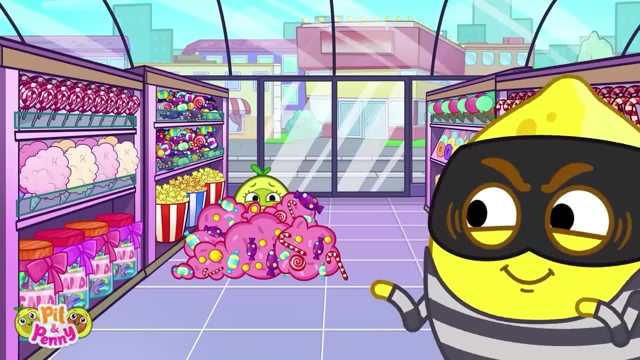 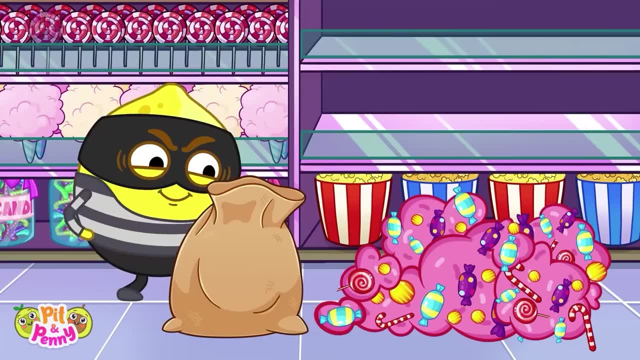 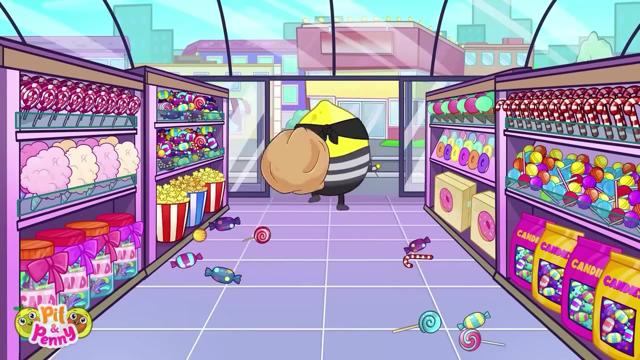 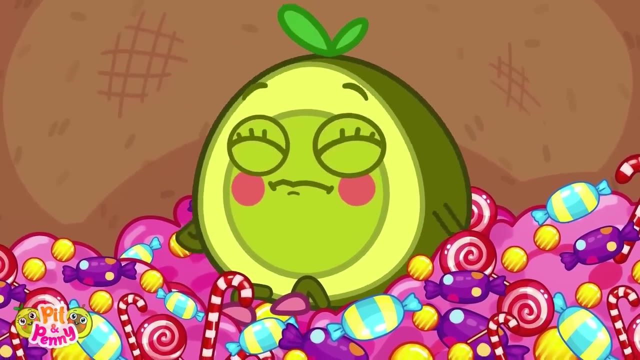 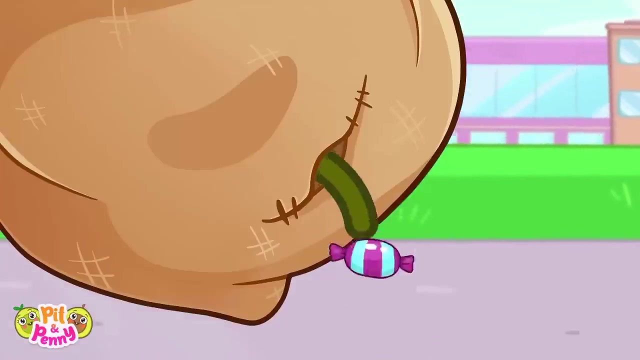 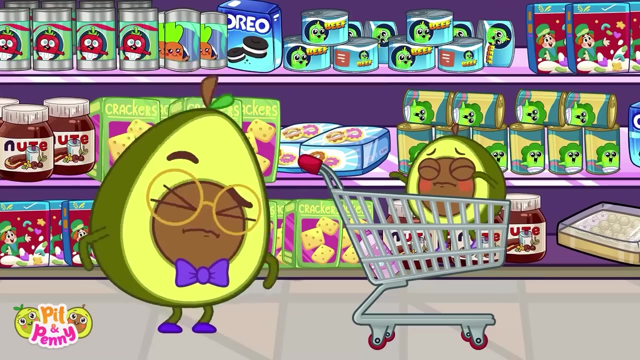 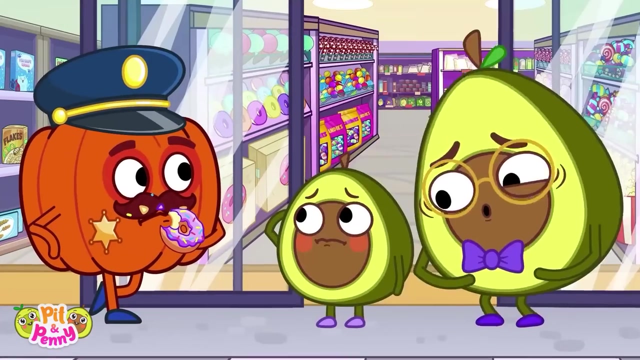 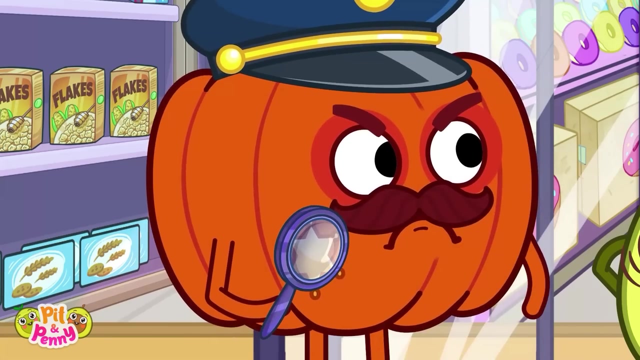 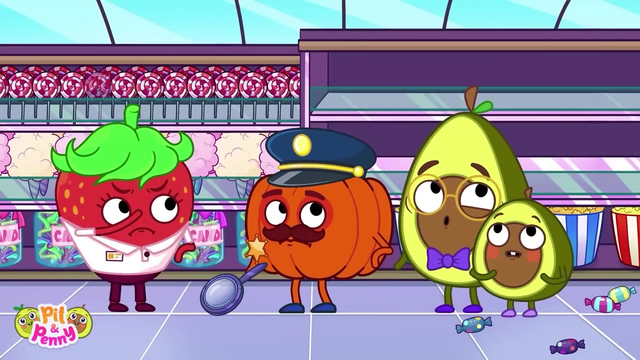 Hahaha. He wants to steal all the candy. Hide Penny. What will you do, Penny? Penny is leaving a trail of candy behind her. How smart. Where's Penny? Maybe Officer Pumpkin can help Penny's missing. What do you think, Officer? 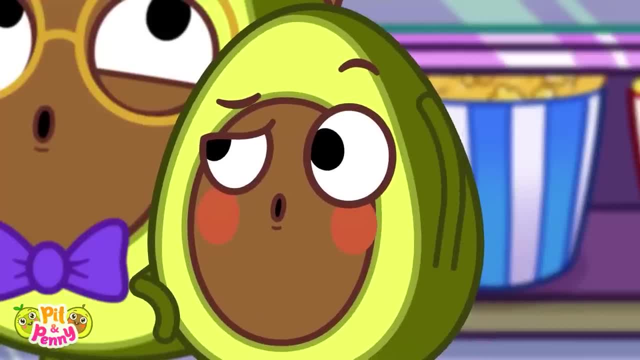 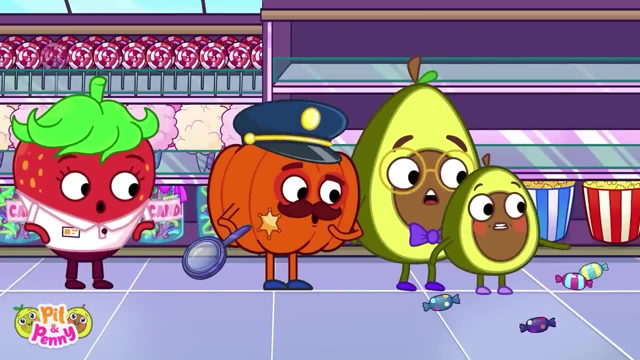 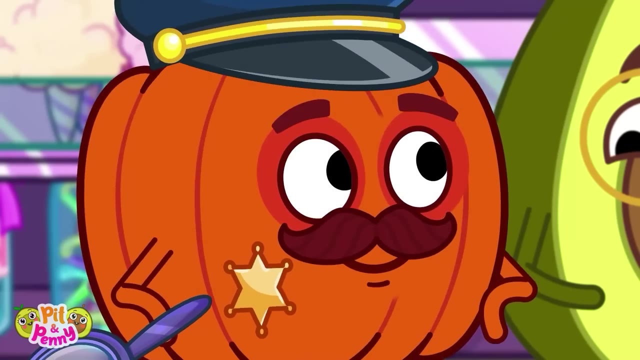 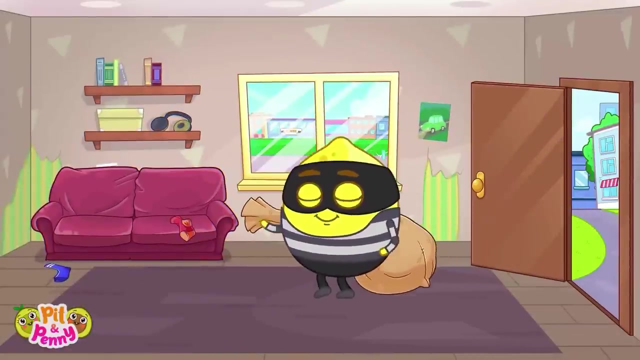 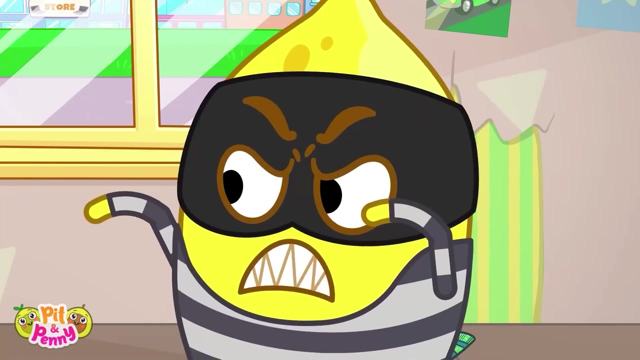 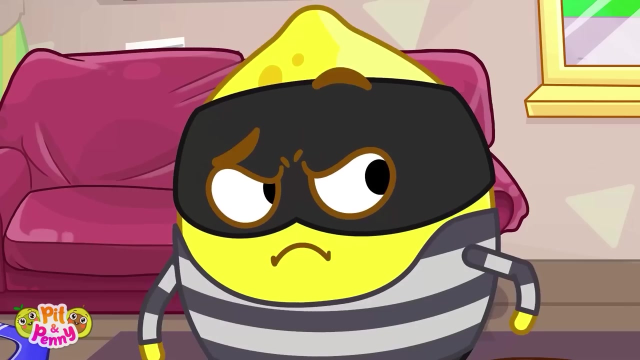 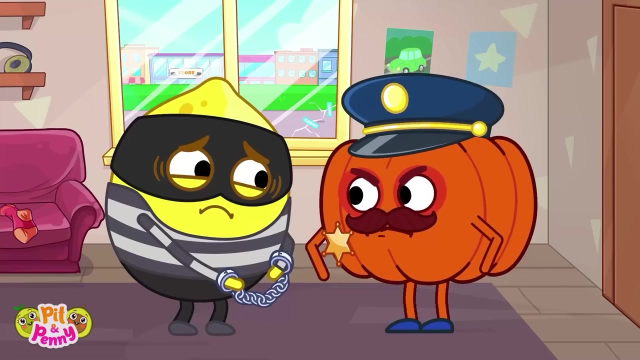 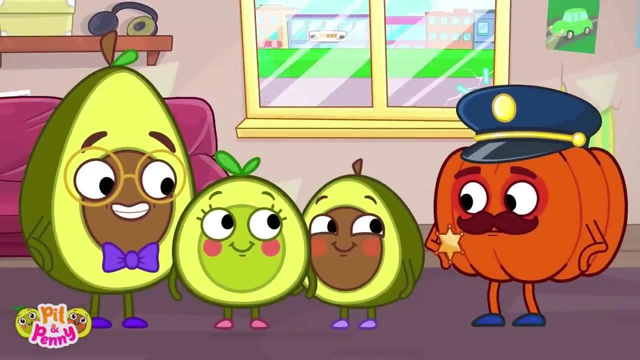 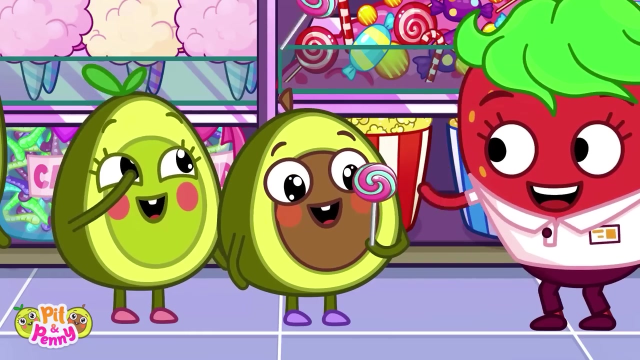 It was a candy thief, Dad. There's a candy trail here. This trail will lead us to Penny. Let's see where it leads. Watch out Penny. It's Officer Pumpkin. Thank you both for your help. Here's a reward for helping catch Mr Lemon. 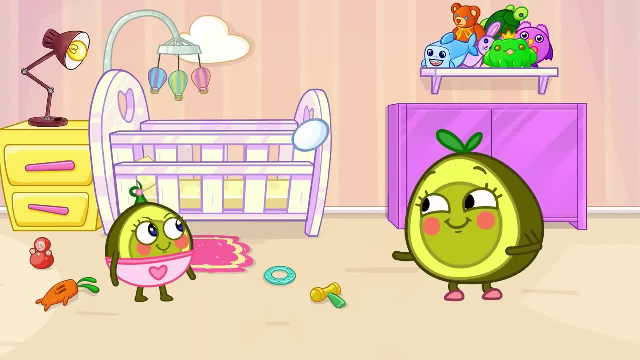 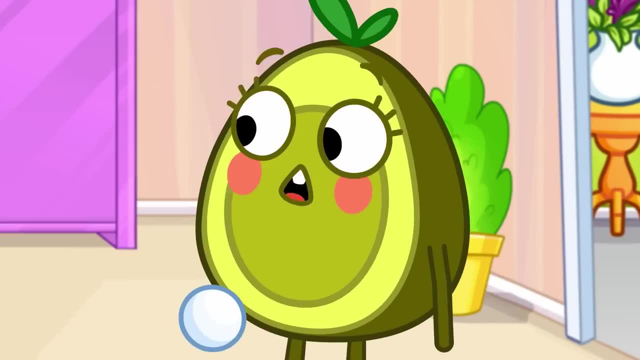 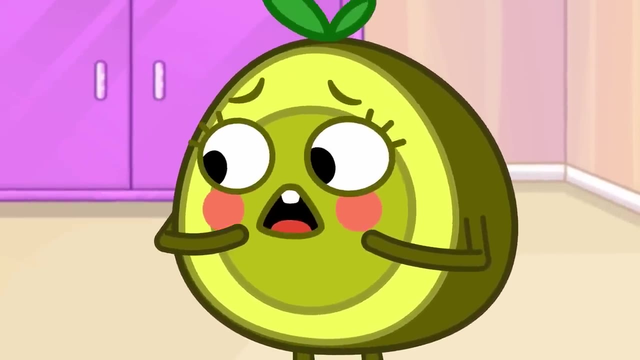 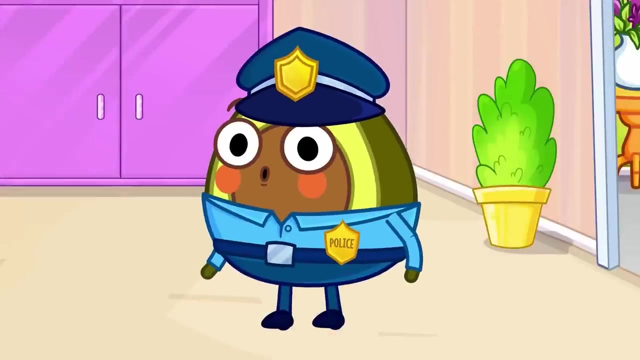 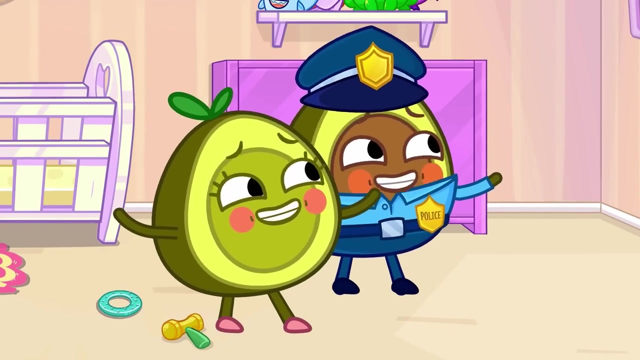 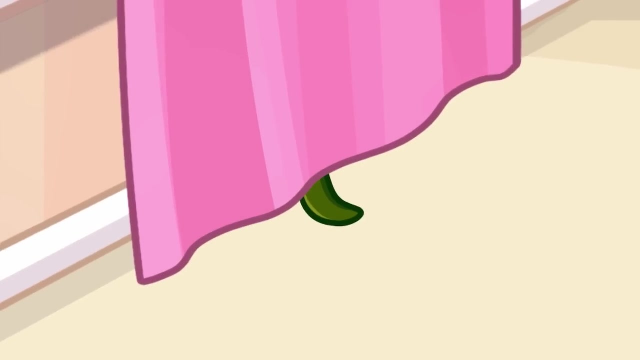 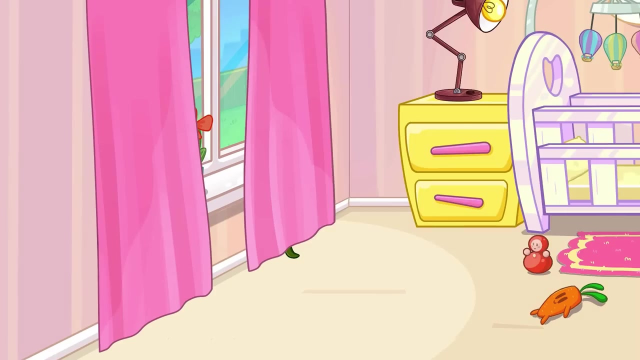 Penny is playing with Baby. Where did Baby go? Oh no, I've lost the baby. Can you help Pit? We will find the baby. Is everything okay, kids? Now let's find Baby. Is she behind the curtain? No, it's just a plant. 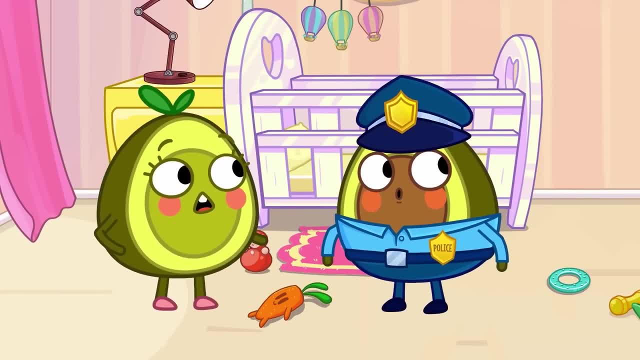 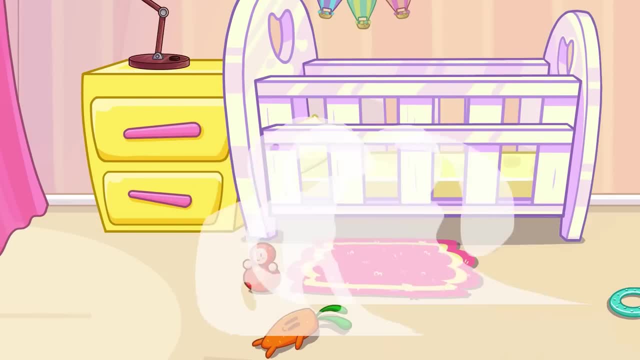 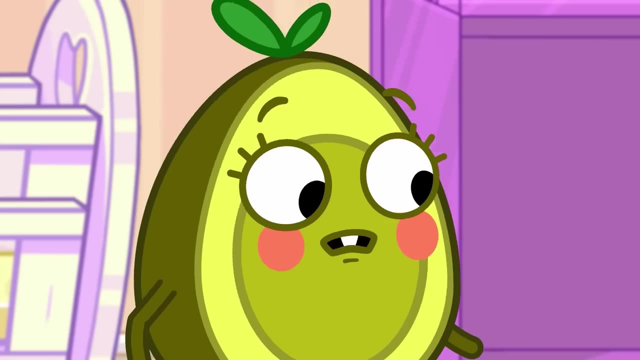 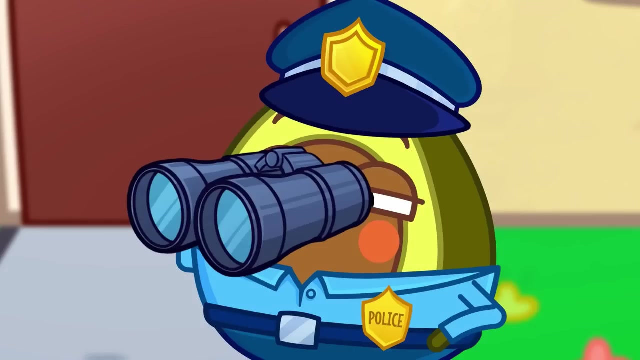 Is that Baby giggling in the cupboard? You should have known. Go and look. You should have known. No, it's Baby's giggle doll. Maybe she's outside in the yard. Could she be in the stroller? Hmm, oh. 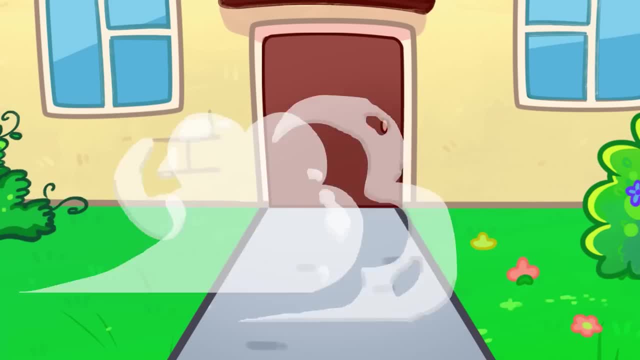 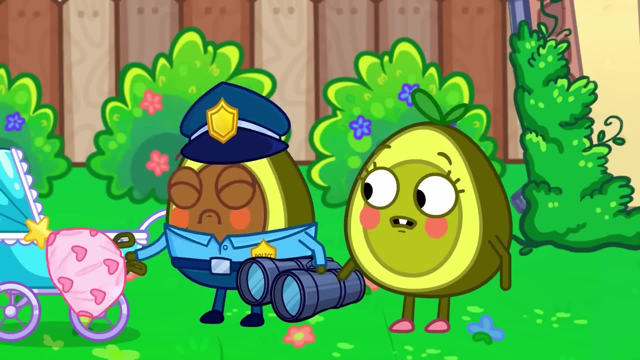 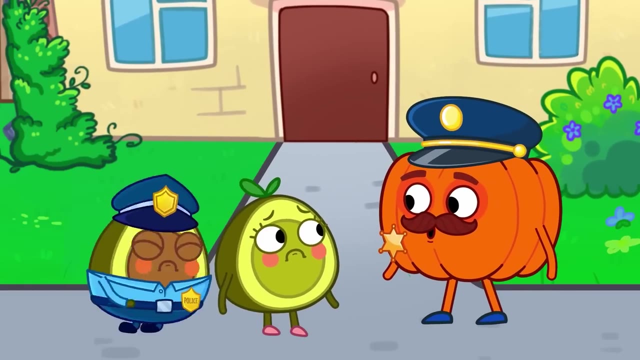 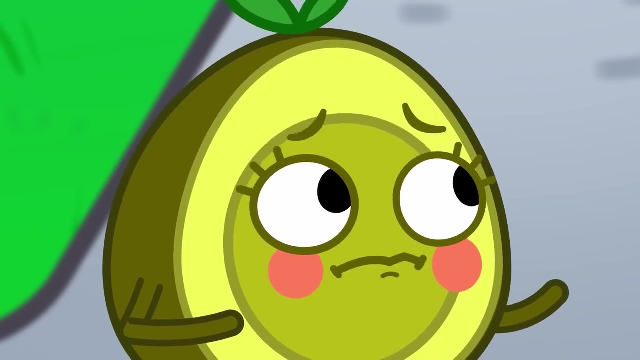 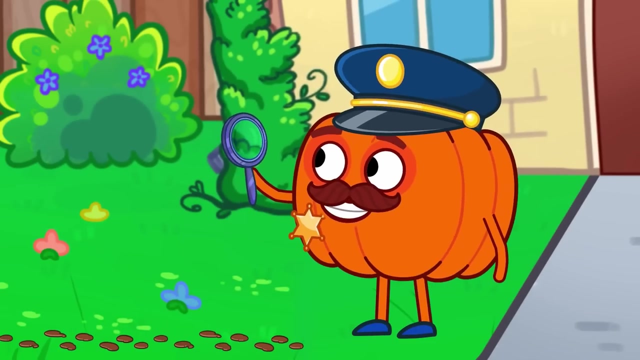 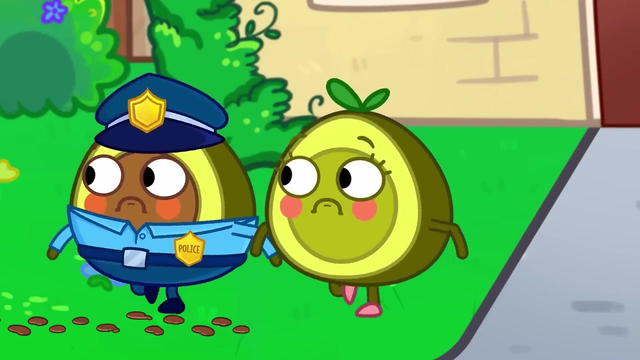 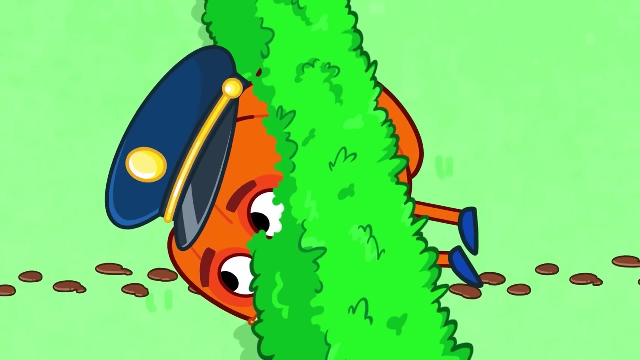 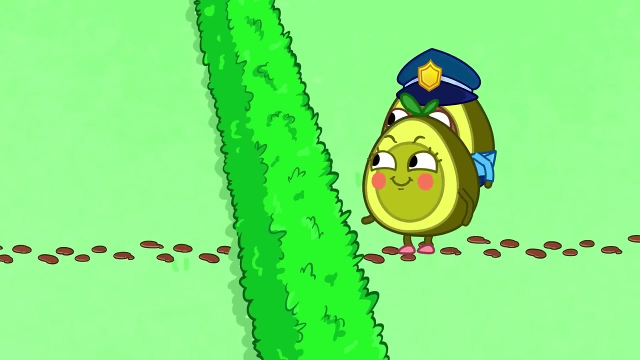 Yes, It's just a bag. Officer Pumpkin can help. We have lost the baby. Officer Pumpkin will look for clues, Footprints- They might lead to baby. There are bushes in the way And Officer Pumpkin is stuck. The footprints lead in there. 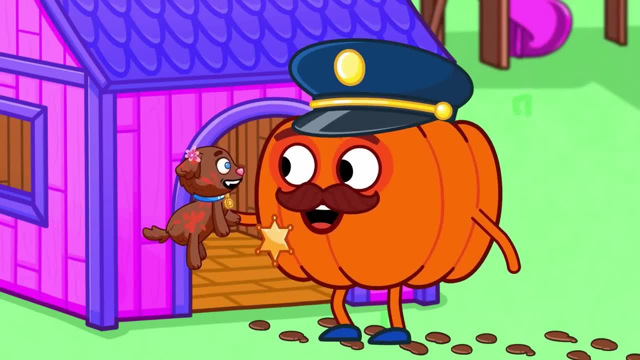 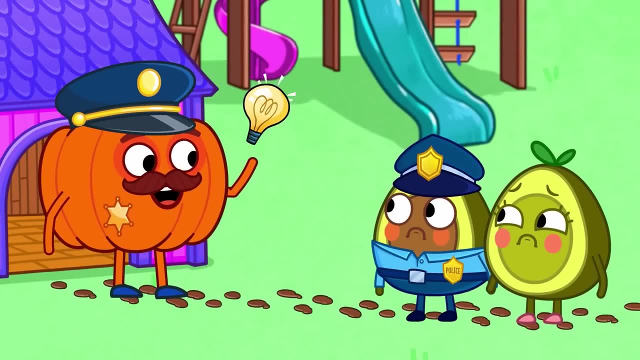 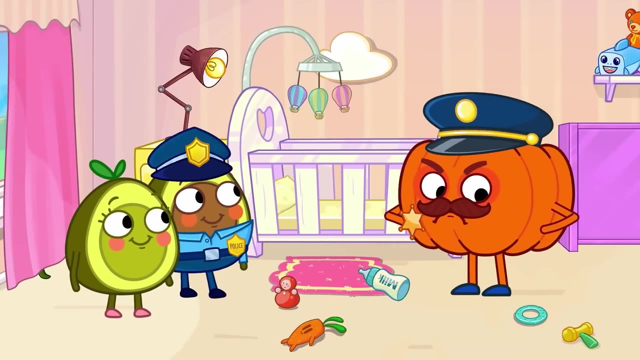 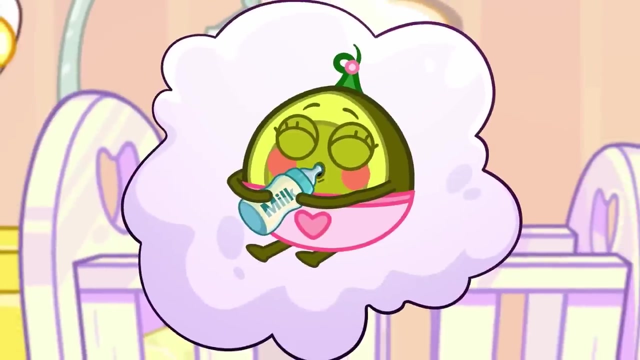 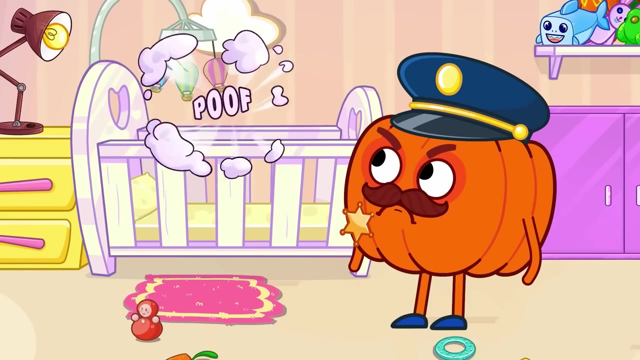 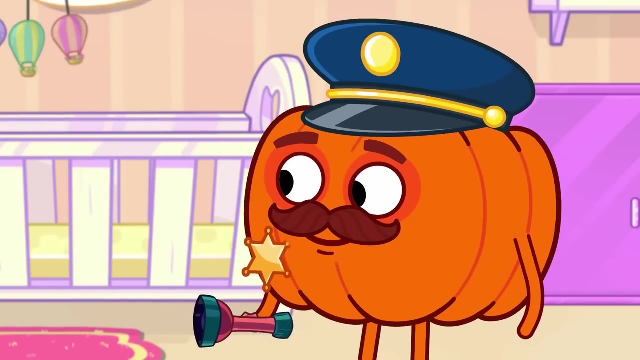 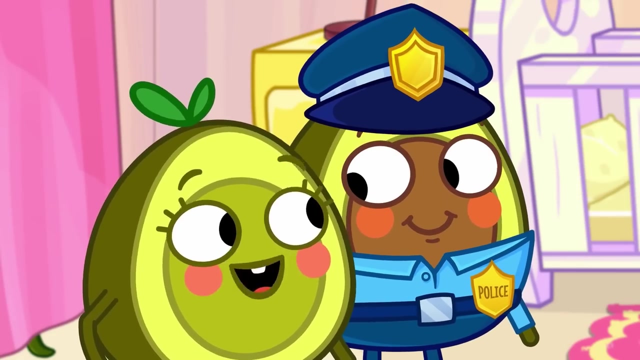 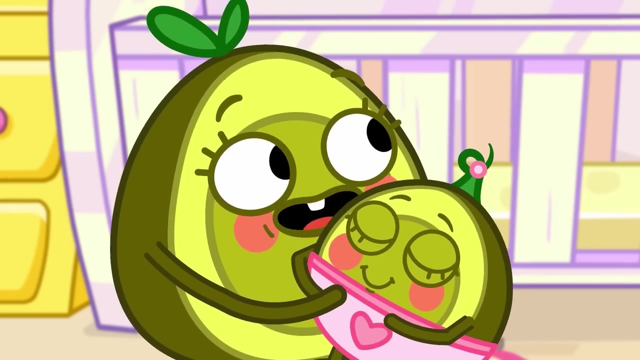 That's not baby, It's a puppy. Let's check it home. Another clue: Baby was in here recently. Follow those footprints. She's sleeping under the crib. Baby has been here all the time. Thank you very much. There's only safe places to play. 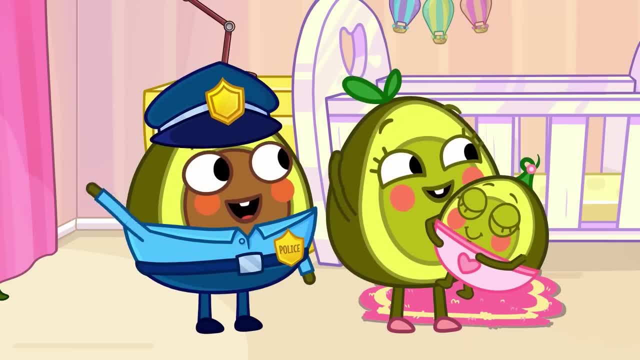 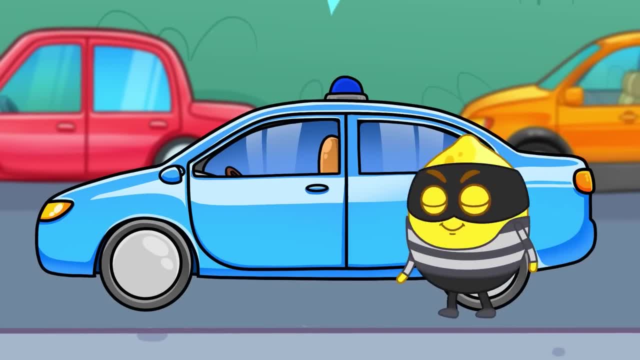 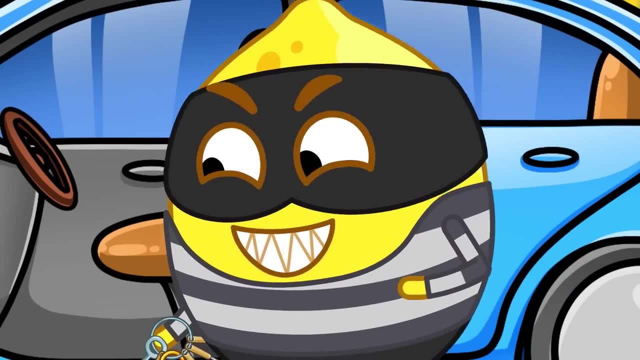 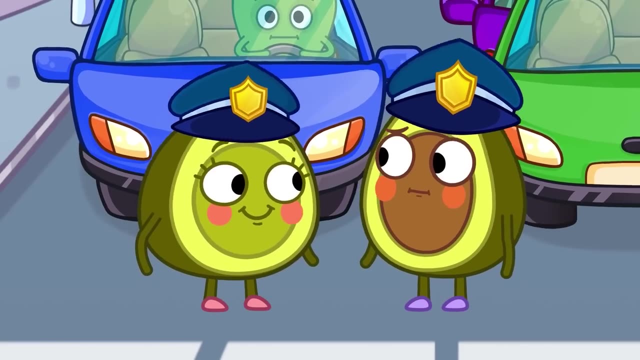 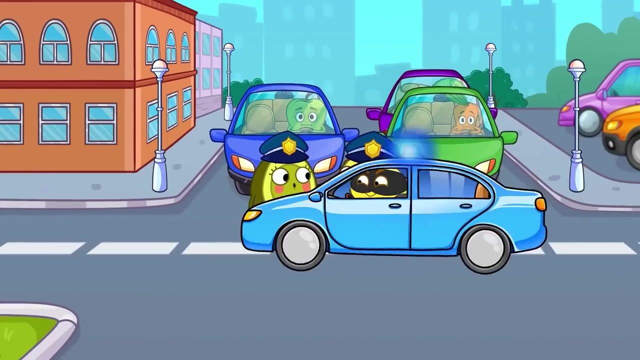 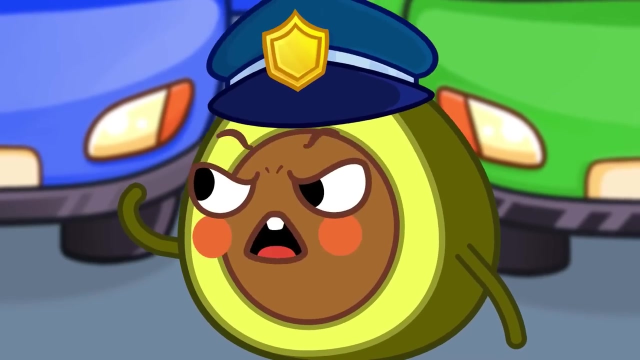 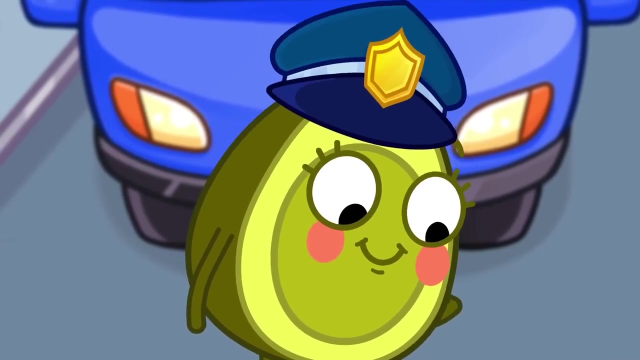 Pit is helping too. Oh no, It's Mr Lemon And he's stealing a police car. The ducklings are safe, Mission complete, But Mr Lemon stole your police car. We need to catch him. Penny knows who to call. 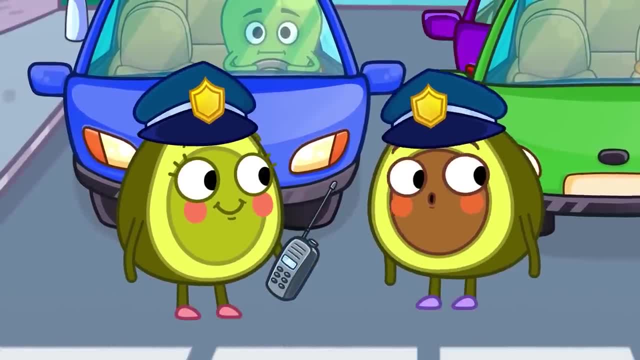 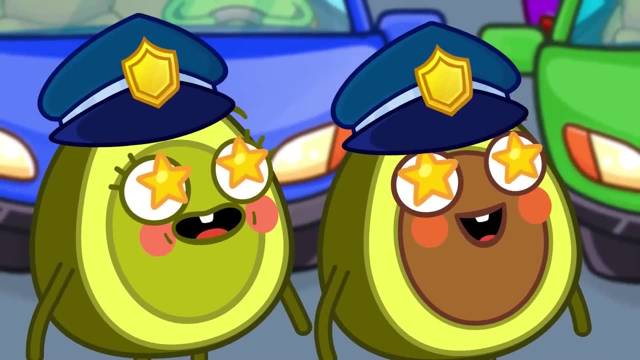 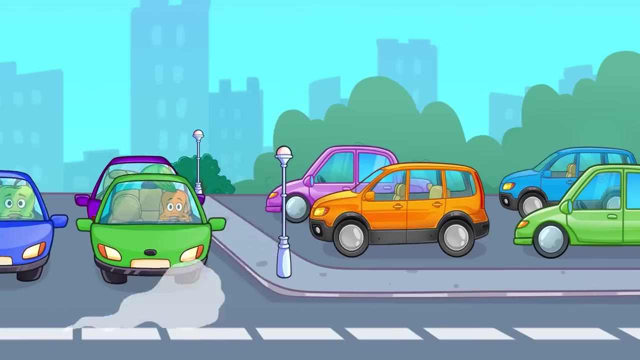 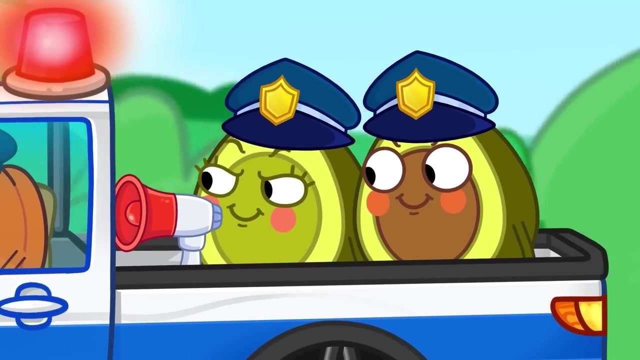 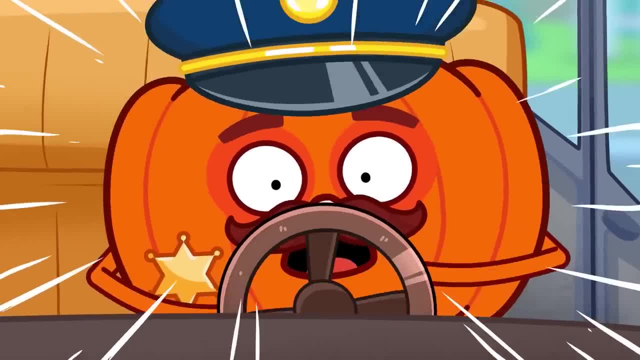 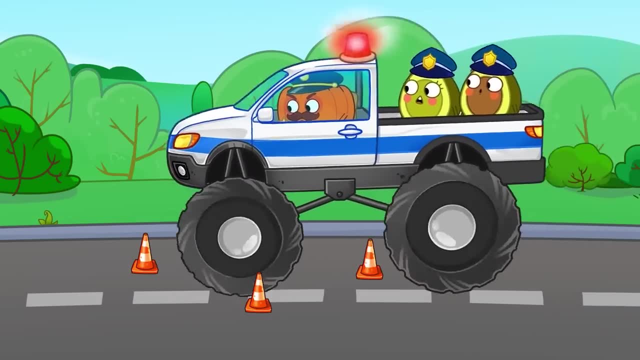 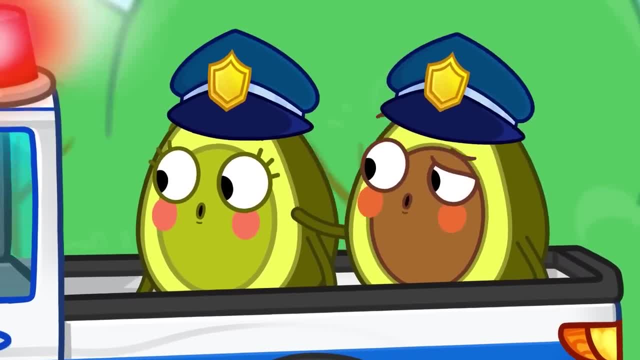 We need some more of these tricks Now. Oh no, Bulgarian rope. Yoless Bear Yesher. He's either running off on a paratrooper. He's either running off on a paratrooper. He's either running off on a paratrooper. 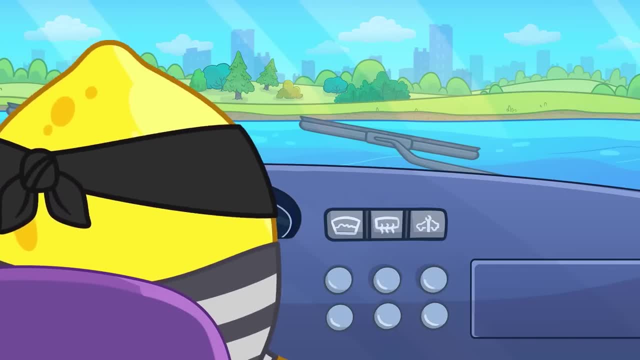 I like this. I like this pair of shoes. Excuse my bad-mouthed miscreant. We find no reason to be afraid. We find no reason to be afraid. Help us make the fight more beautiful. Heп, He'll float across. 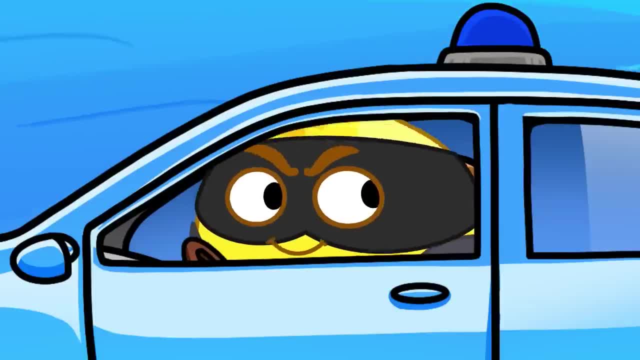 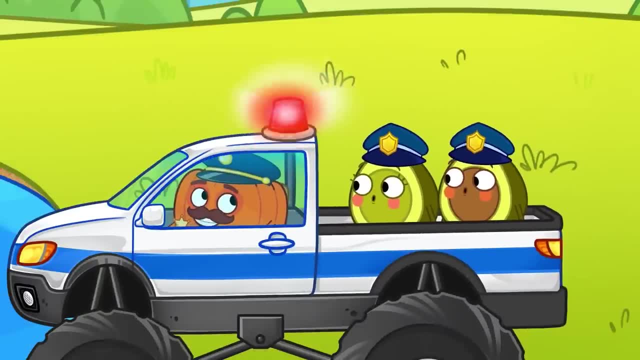 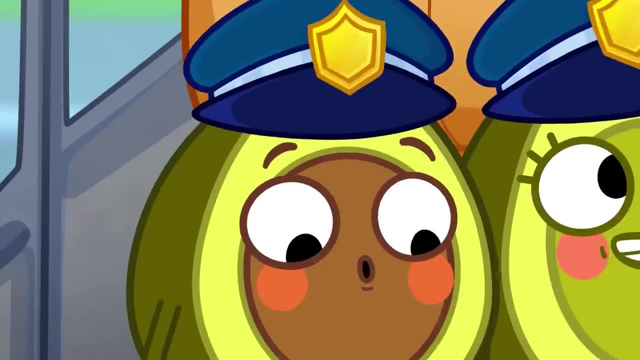 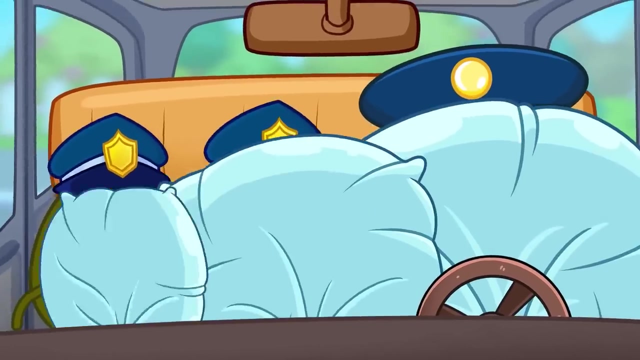 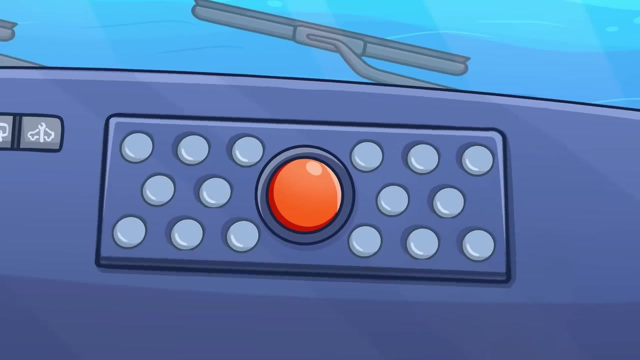 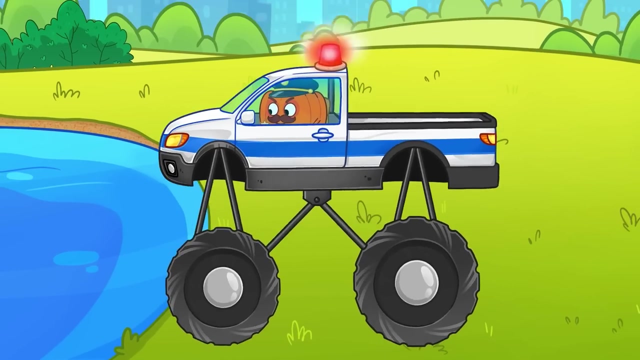 We find no reason to fear. Mr Lemon looks fry Hecap. He gun Heap. Come on, officer pumpkins truck won't? officer pumpkin has a plan. don't hit all the buttons, pitch you. that's better. now the truck can drive across. 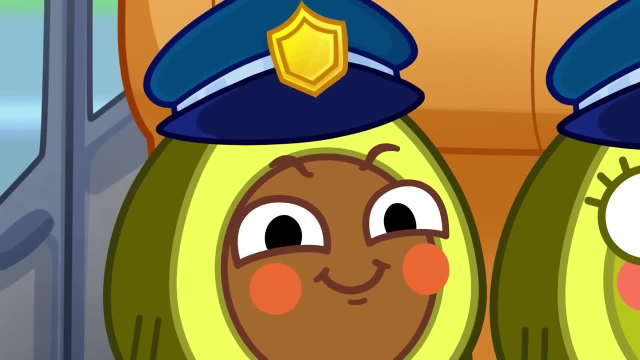 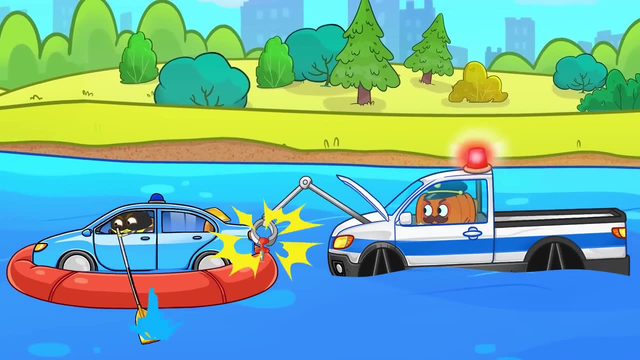 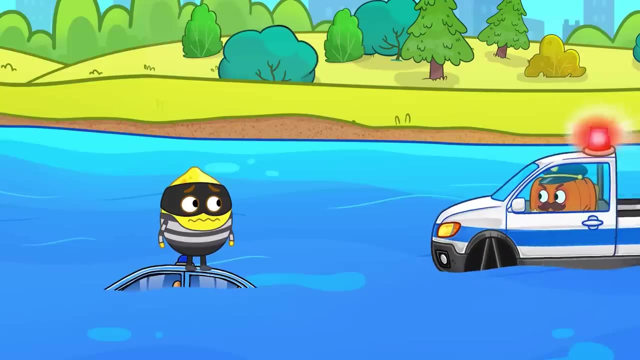 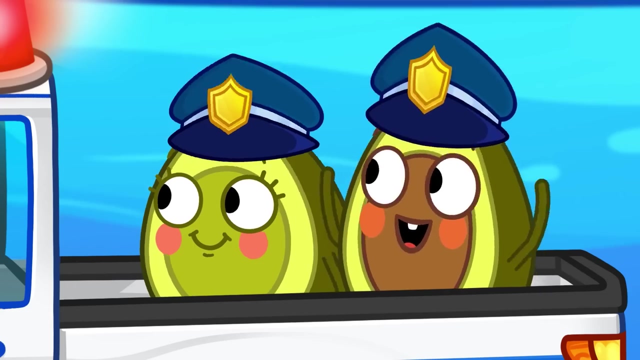 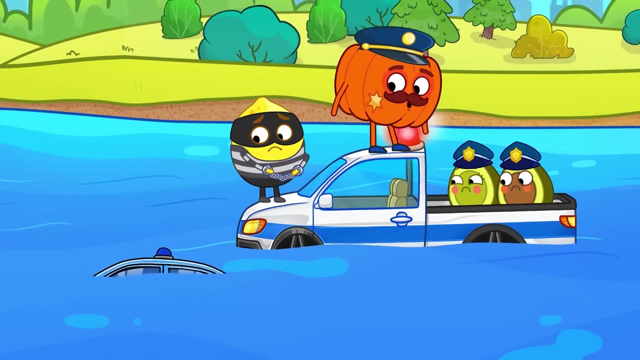 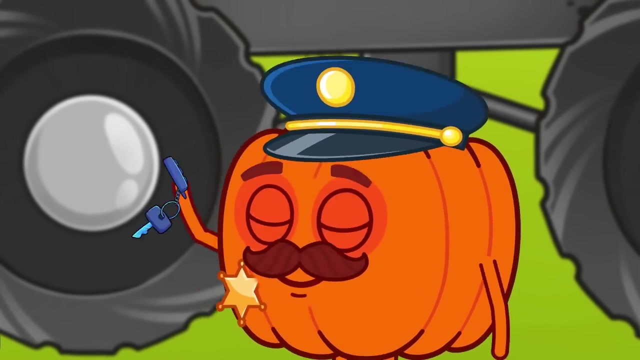 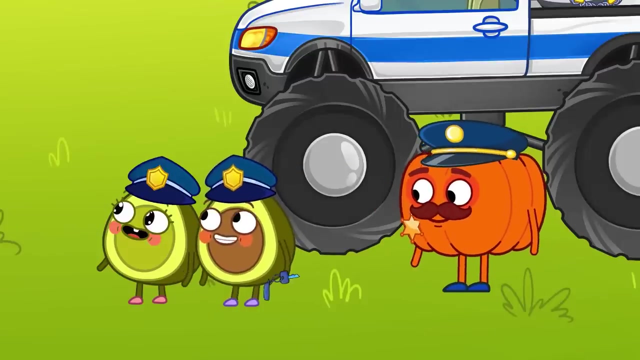 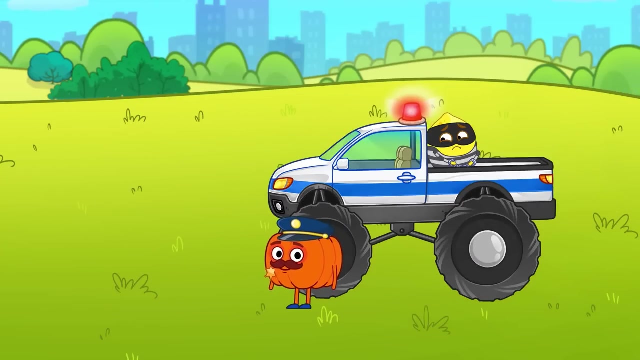 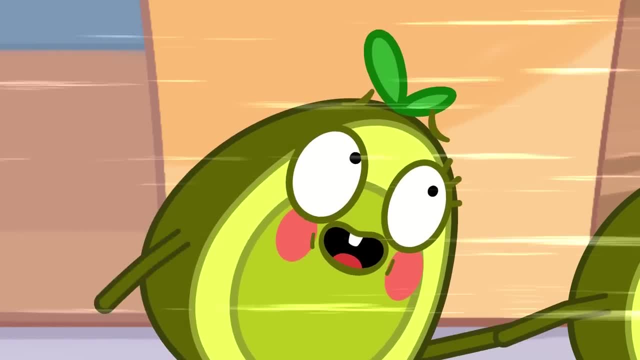 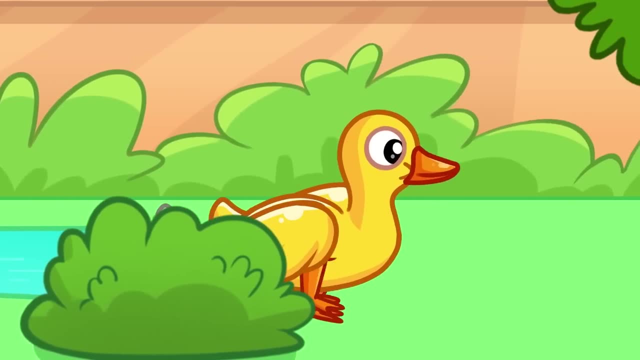 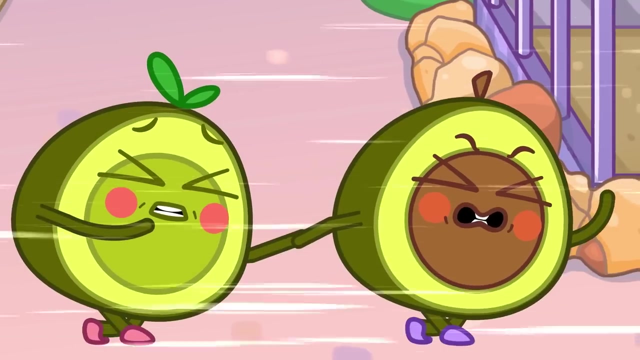 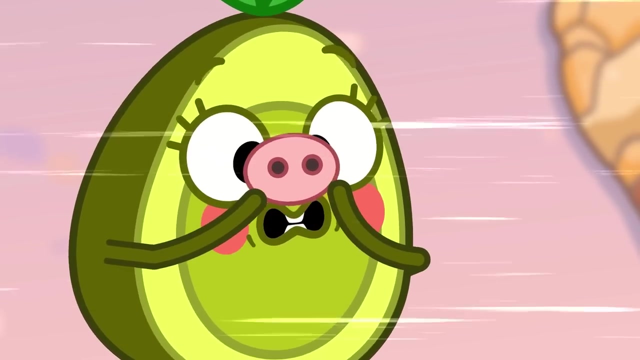 can use. thanks, officer pumpkin. it's can use. thanks, officer pumpkin. it's a very windy day. a very windy day. Oh no, Pig lost a snout And duck lost her beak. It's duck's beak And pig's snout. 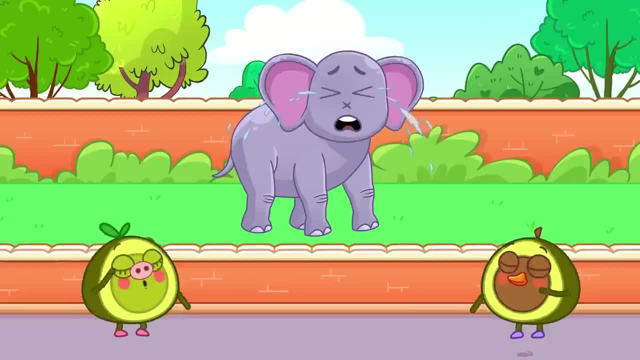 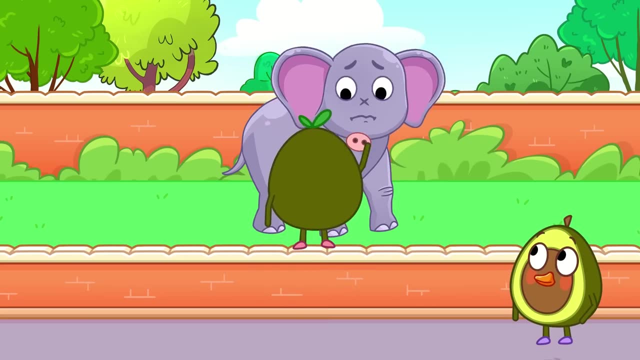 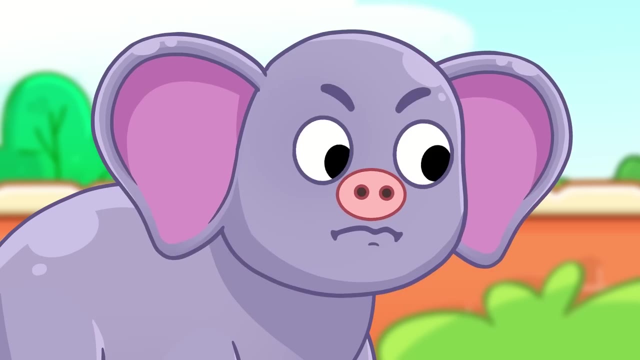 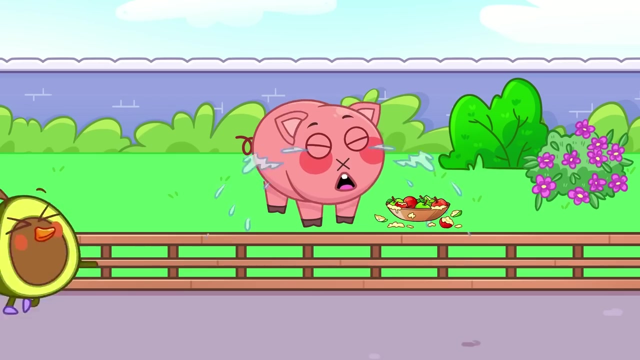 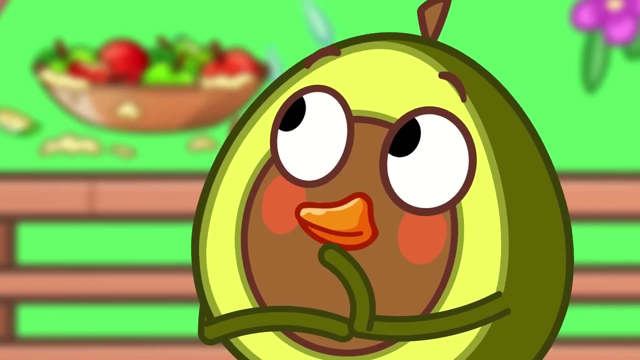 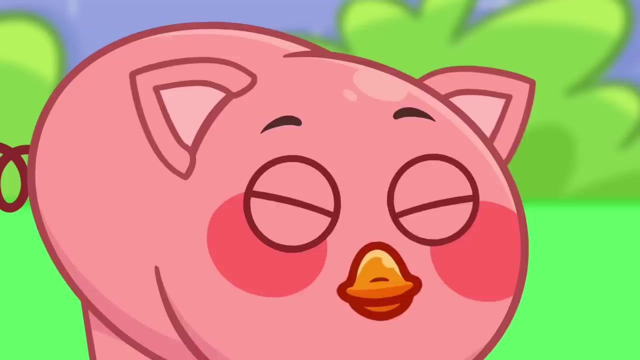 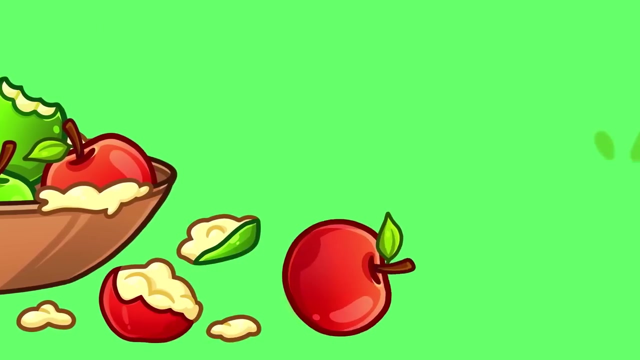 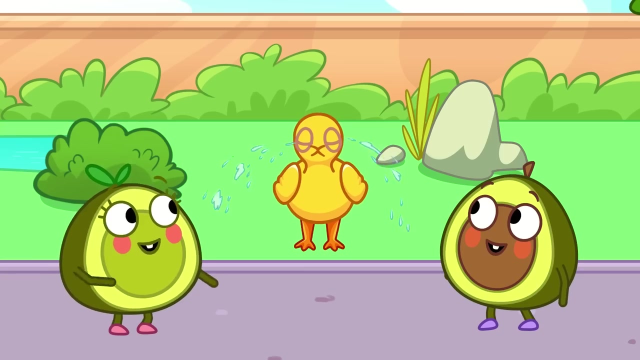 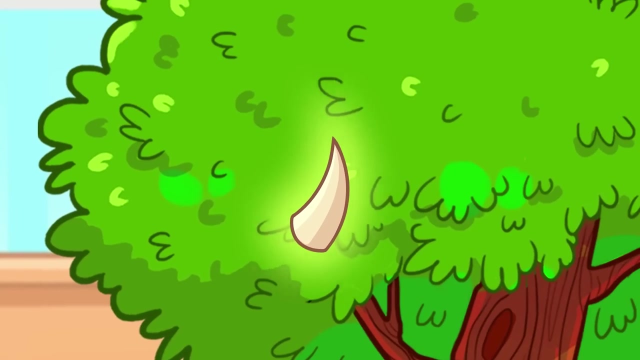 Elephant is crying. He lost his trunk. But, Penny, that nose belongs on the pig. But Pit, that nose belongs on the duck. Duck is missing her nose as well. What do you see, Penny? A rhino horn, A rhino horn. 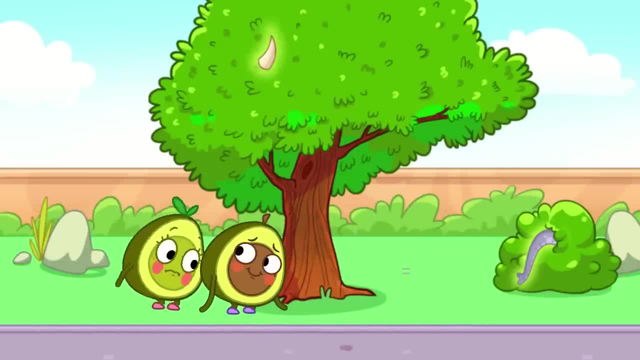 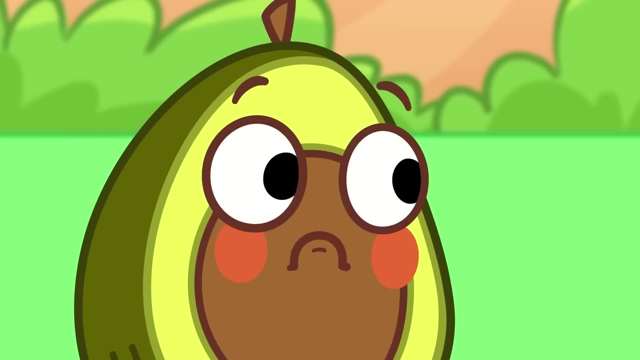 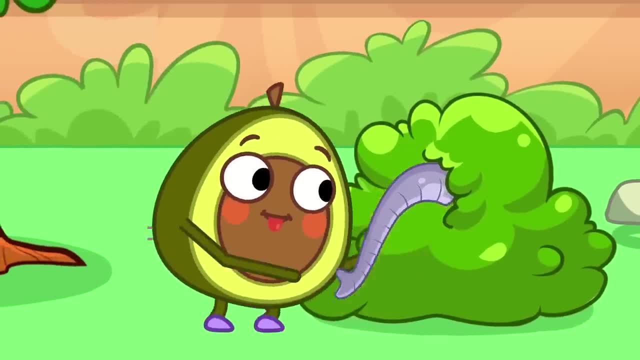 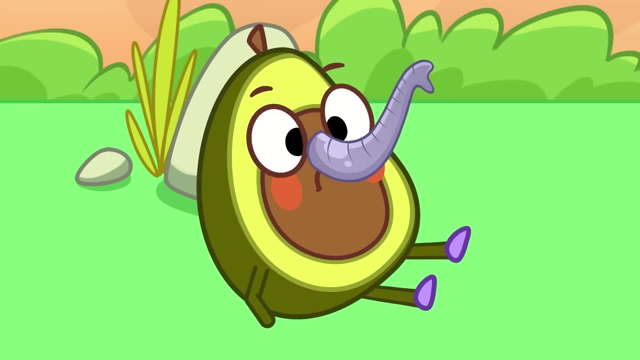 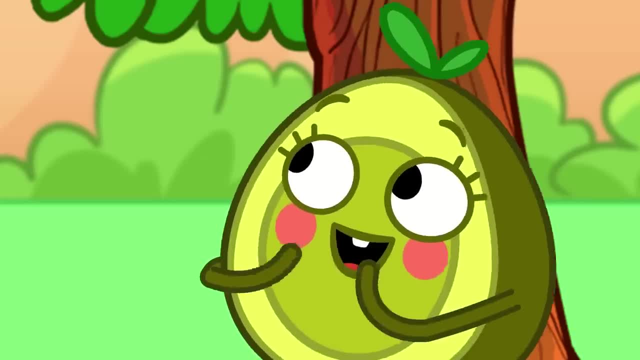 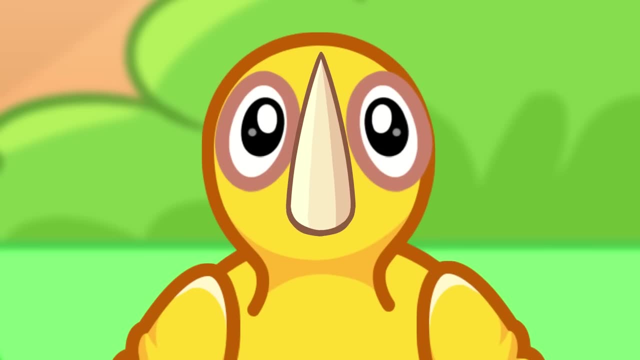 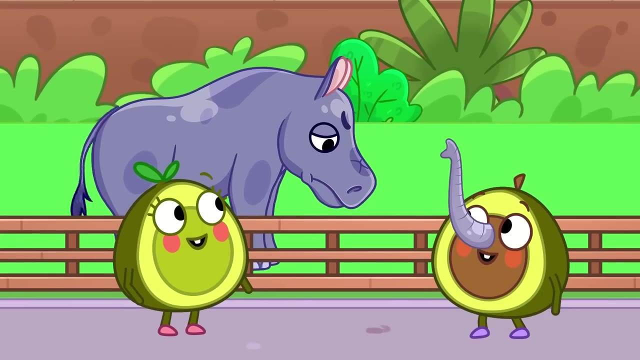 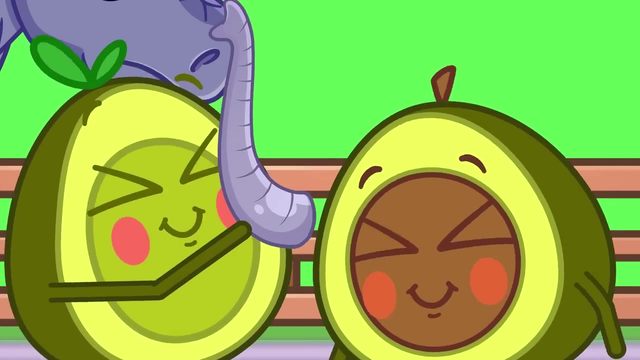 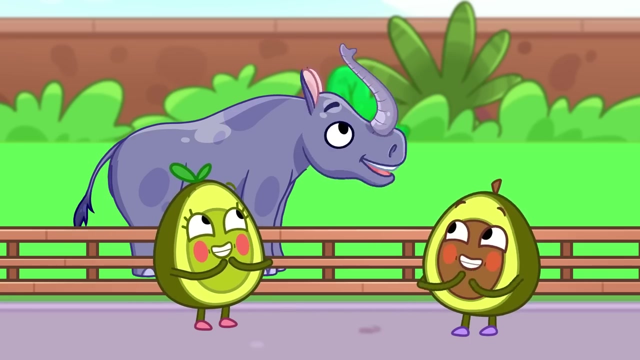 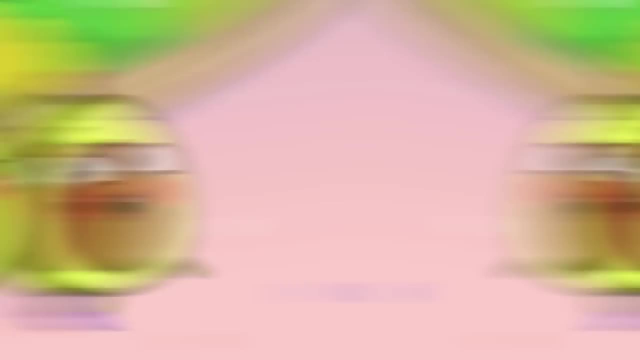 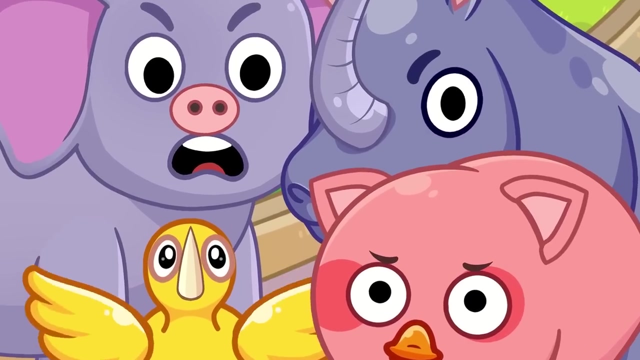 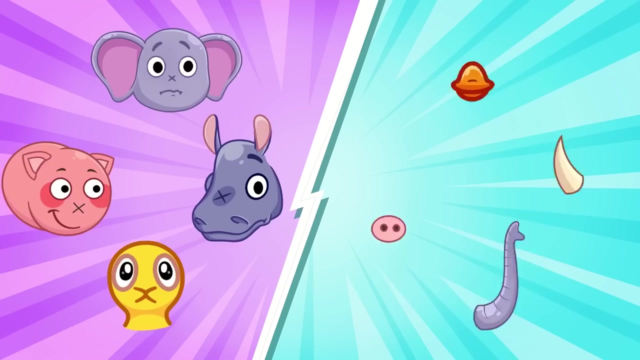 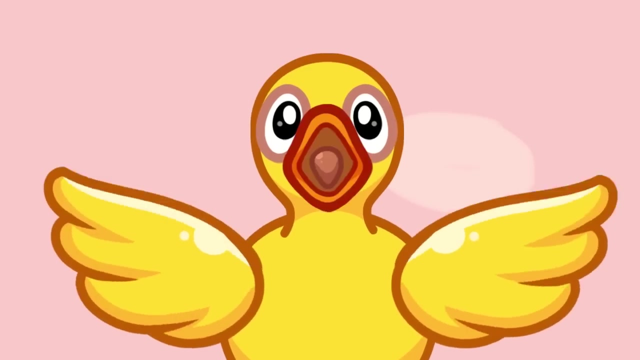 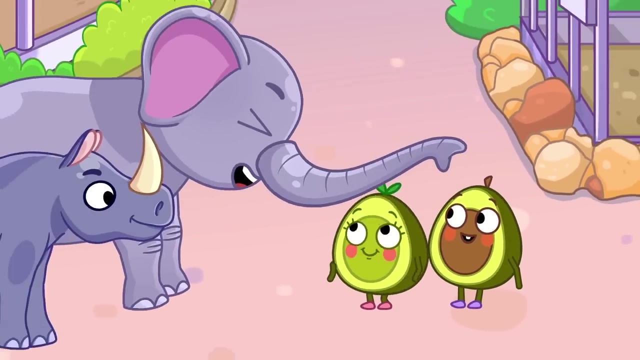 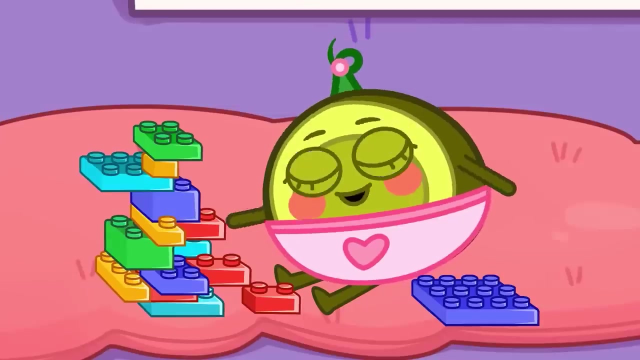 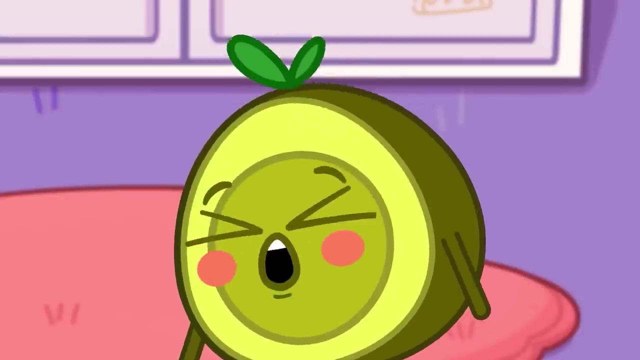 The animals want their proper noses back. You can do it: Pit and Penny Pig has his snout, Duck has her beak, Rhino has his horn And elephant has his trunk. Well done, Baby is playing with building blocks. What if she becomes a builder? 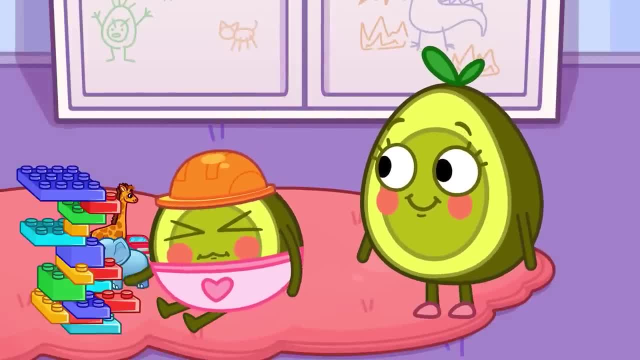 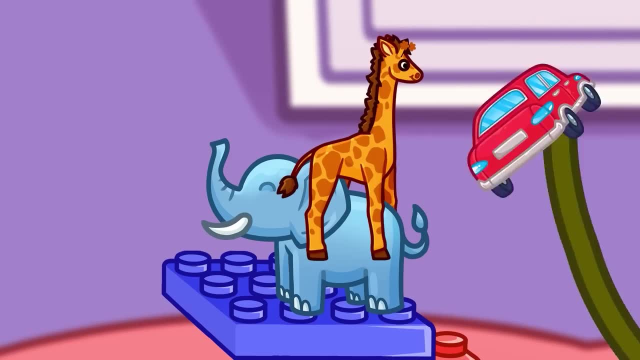 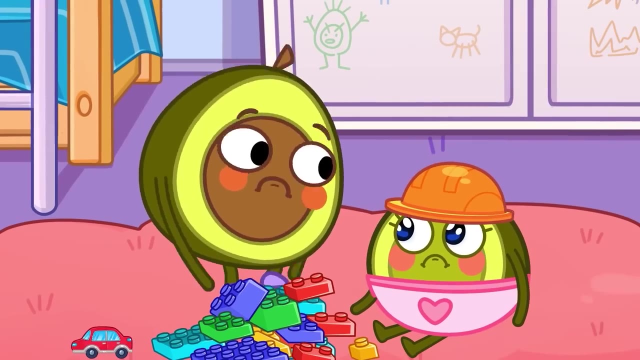 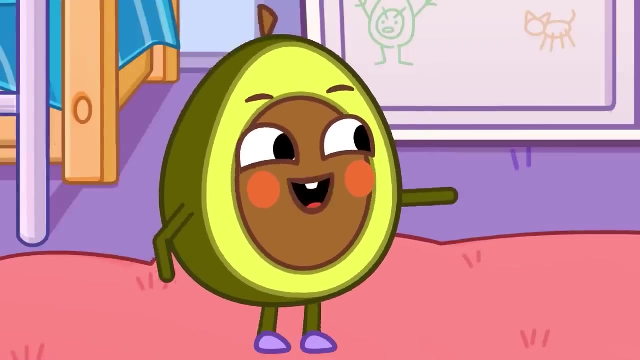 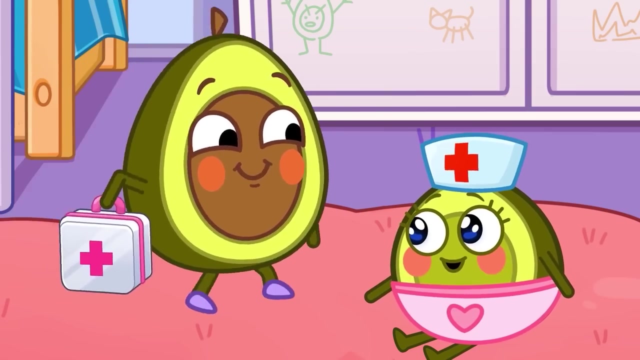 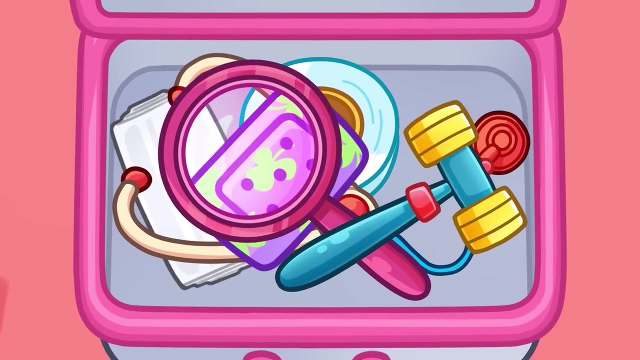 Would Baby be a good construction worker? Uh-oh, That building is going to fall. Pit thinks Baby needs a different job. No, She will become a doctor. Doctors help people when they're sick. Look at all the things she can use. 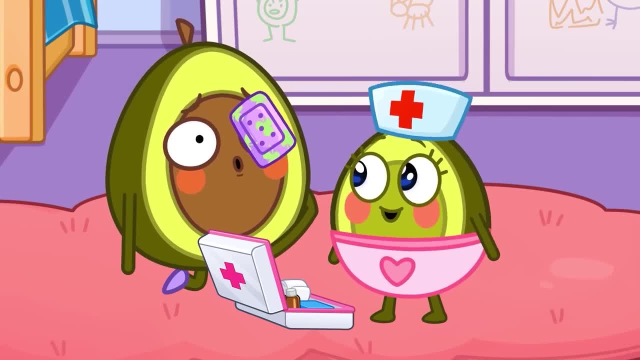 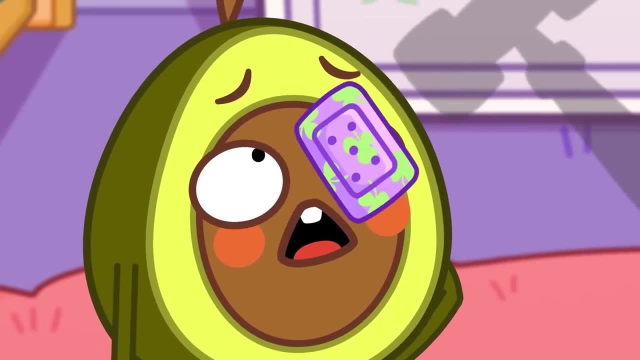 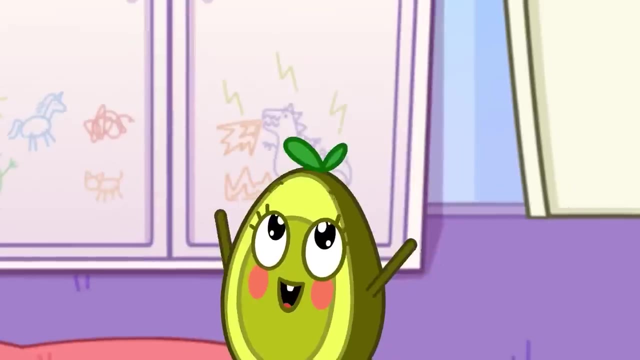 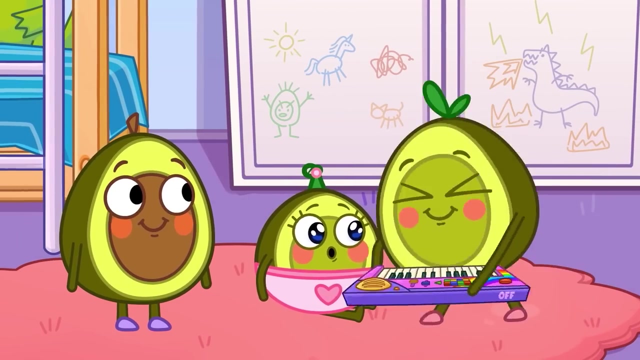 Let's put a bandage on Pit. That isn't the best spot for one. Now she has a little hammer. Penny, can you think of something else for Baby to do? She'll become a musician. Can she play the piano? Give it a try, Baby. 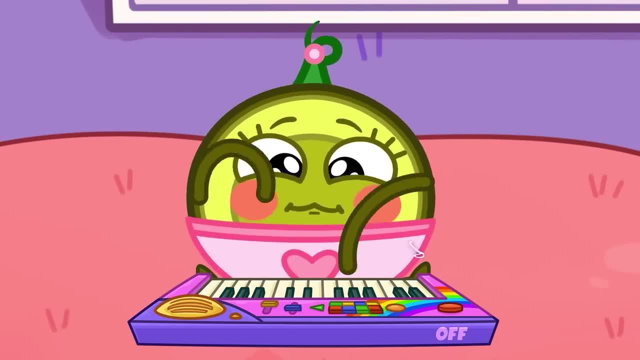 I can do it. Look, she's a piper. That was fun. Oh my gosh, I've never heard much of her play. I can see it. She's an opera singer. I've heard so much about her. She's a big hit. 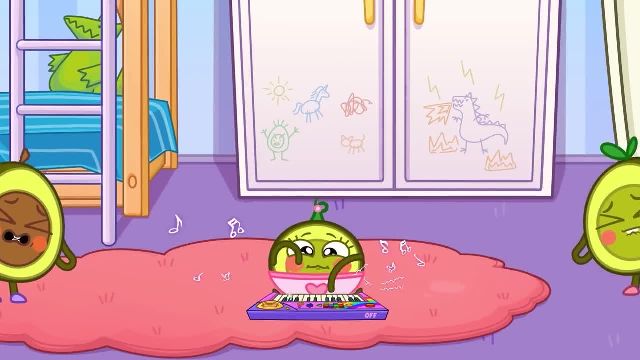 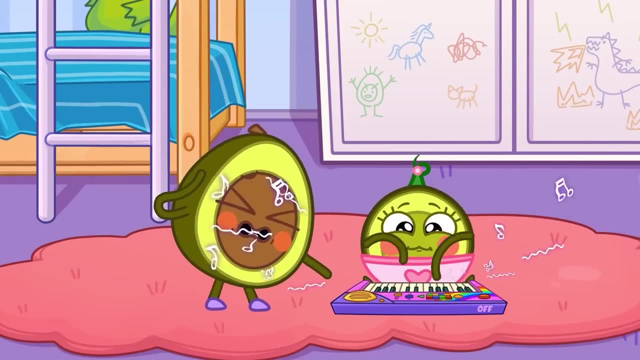 She should be quite popular. You got a big mic baby, You're right, I know Now she can play music. But how Wait, You've already made a million, Can you even make these? I have many, All my babies. 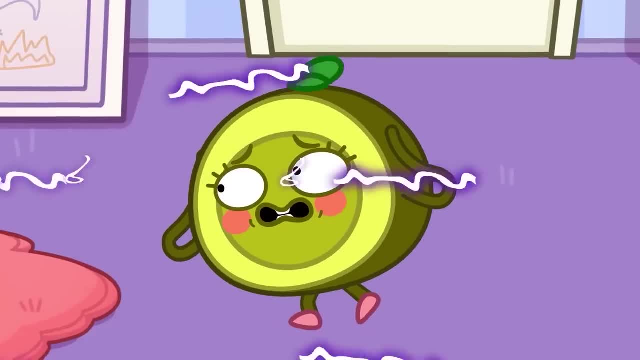 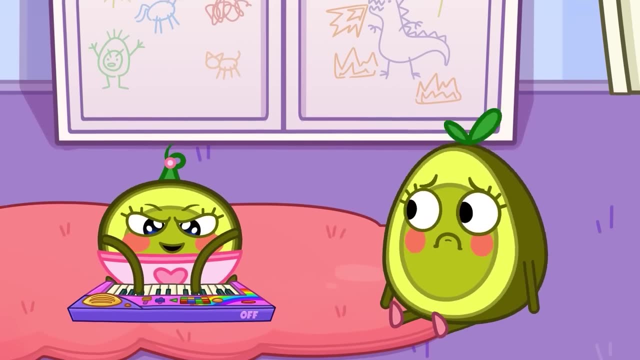 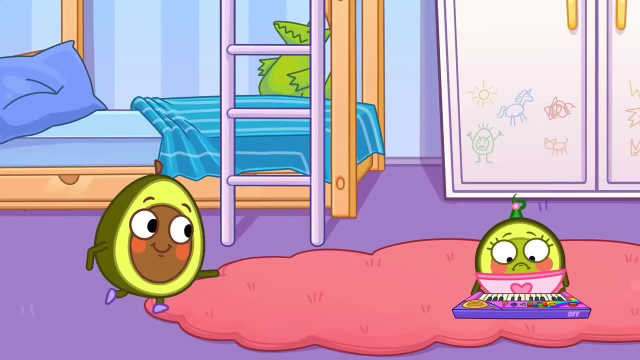 You can make all kinds of music with this. I'll try, I'll try. She's got a big, big heart. Great, Well done. I'm sorry, Penny. I'm sorry, Penny, Phew, that's better. 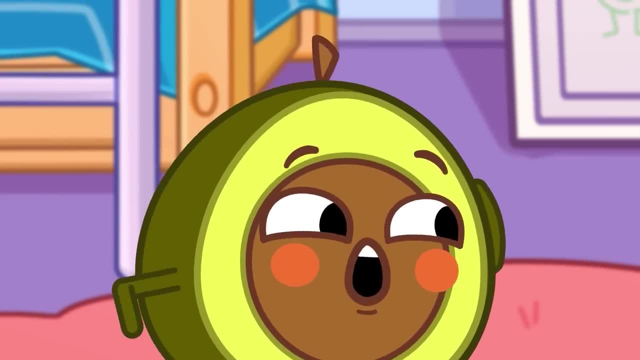 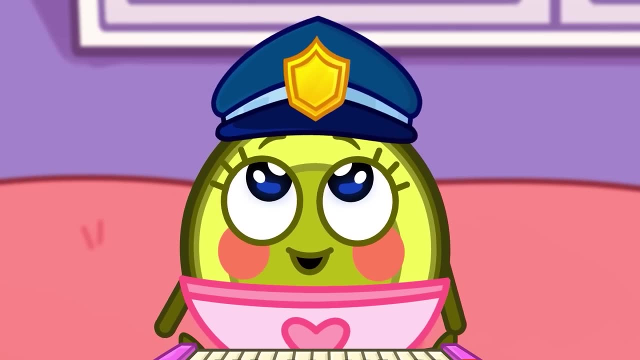 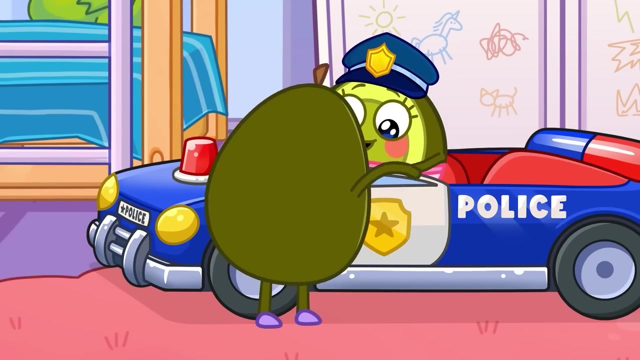 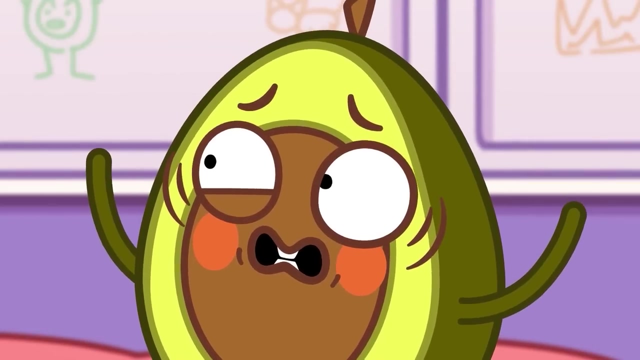 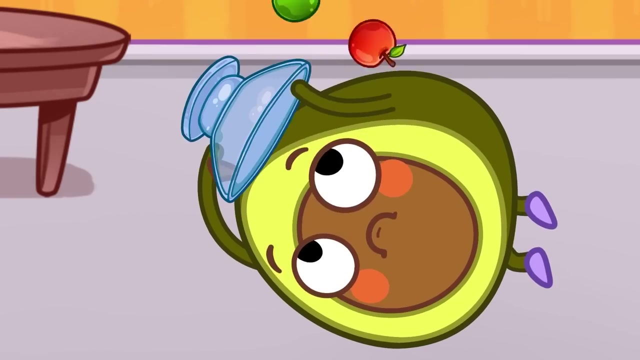 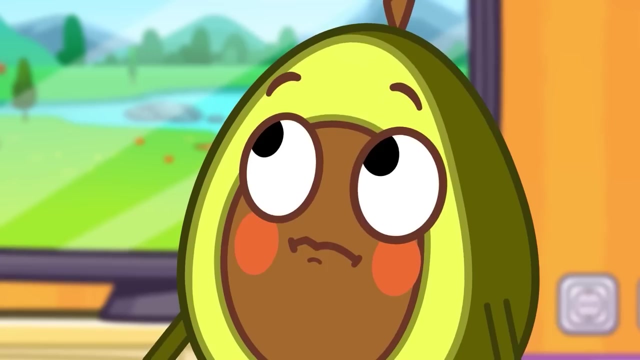 What else can Baby try? She will become a police officer. Police officers: keep people safe. Here's your police car, Baby. Slow down, Baby, or you'll break something. Ooh Pit, saved the TV. Watch out Pit. 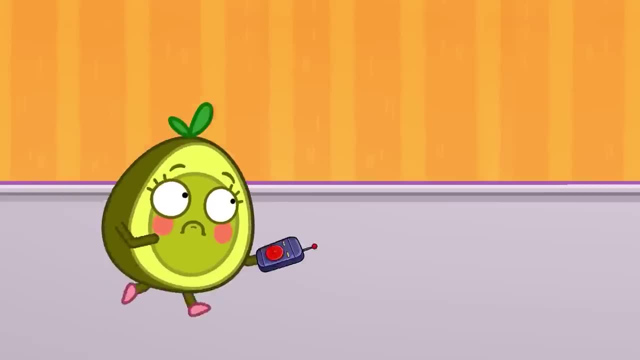 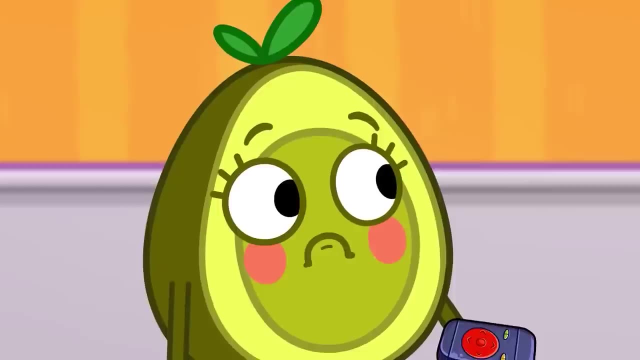 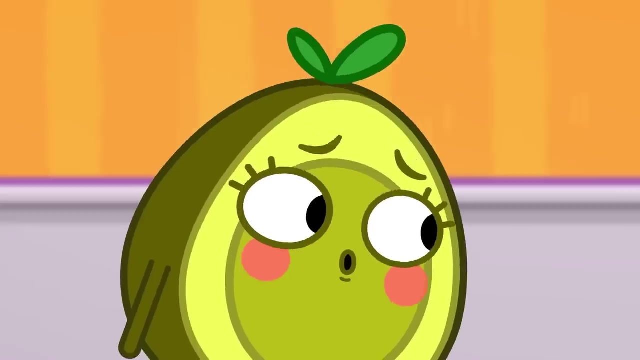 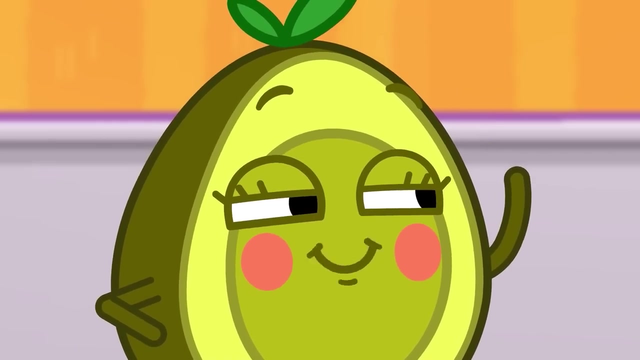 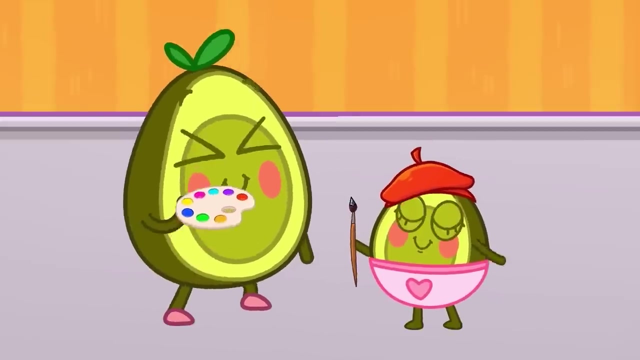 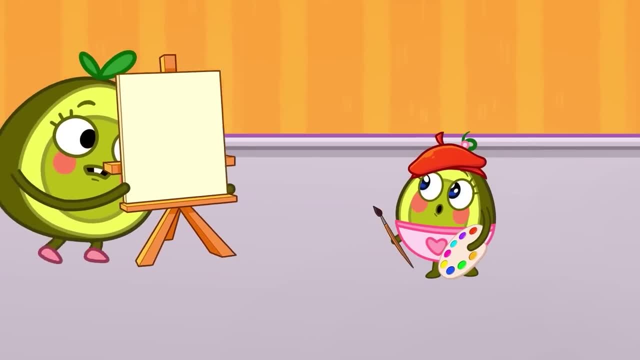 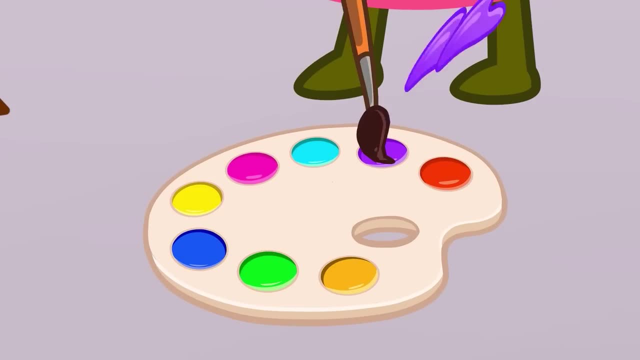 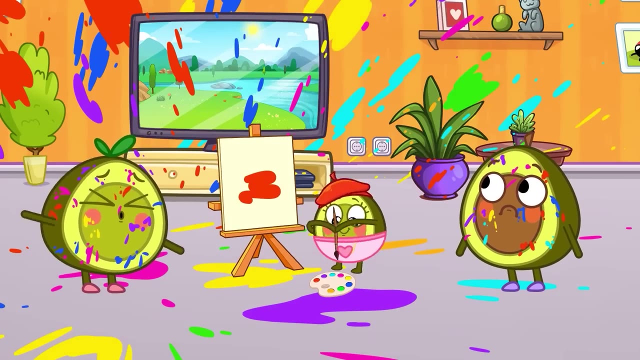 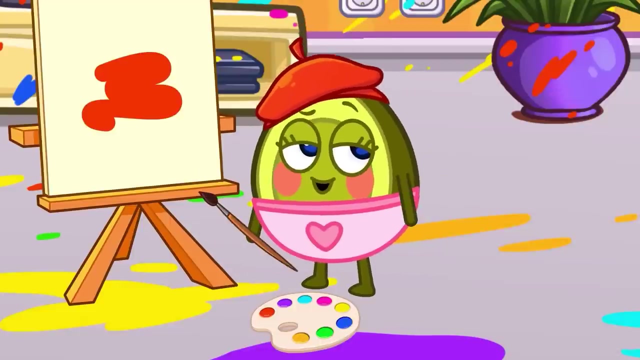 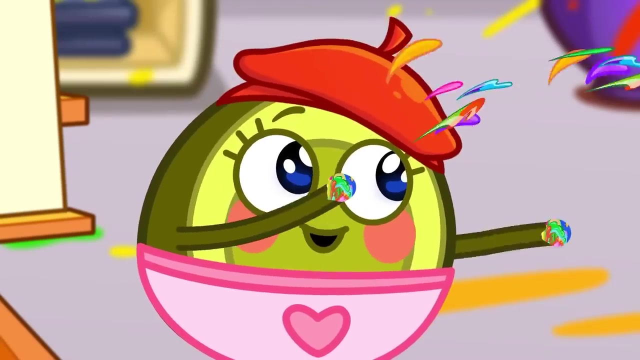 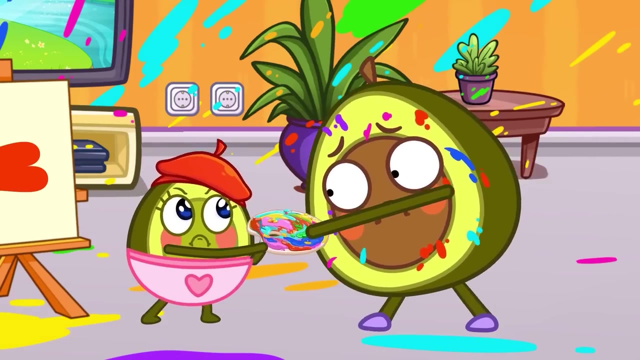 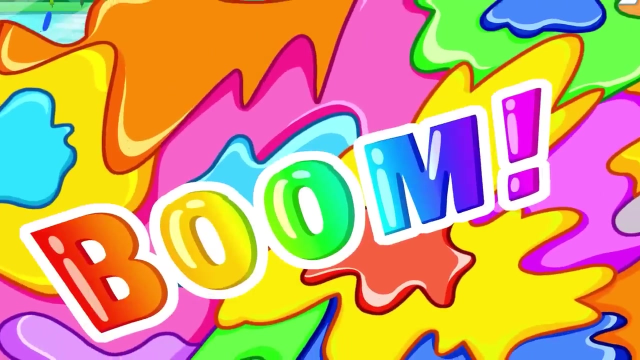 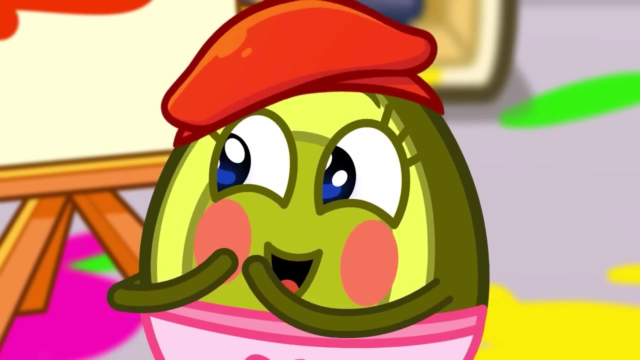 And an easel to paint on. What will Baby make? Baby will make a mess, Oh no, Ah, Ah. Ah. No, baby, You'll get paint everywhere. Maybe being an artist isn't the best choice. Daddy is helping clean off the paint. 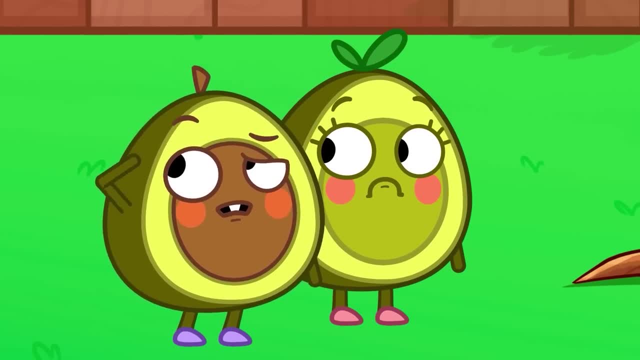 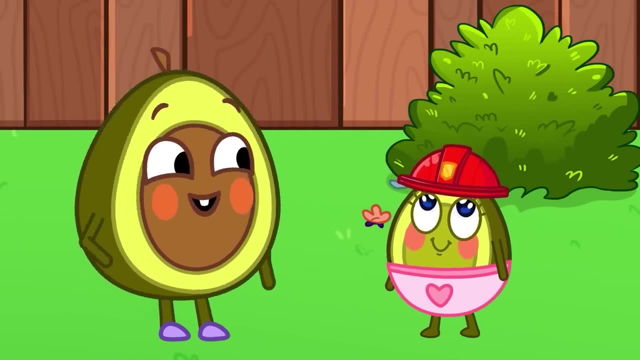 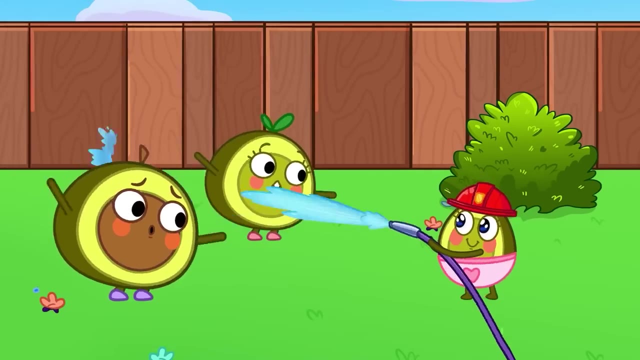 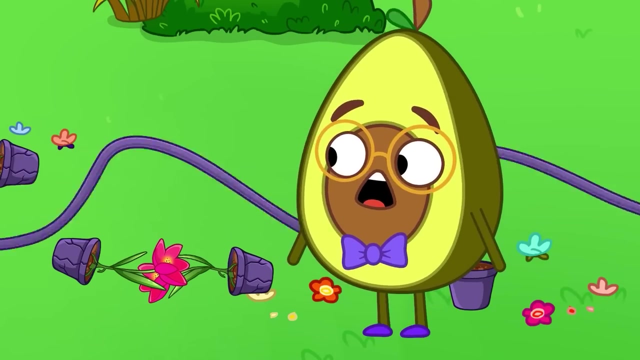 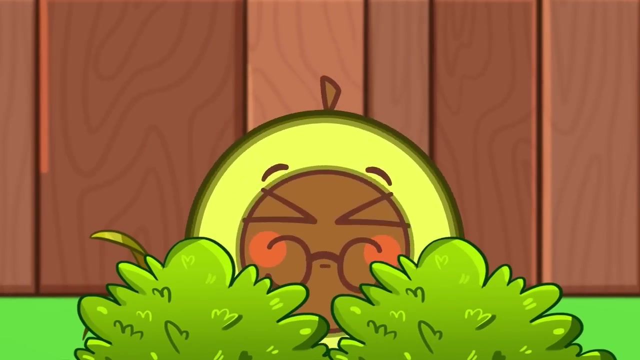 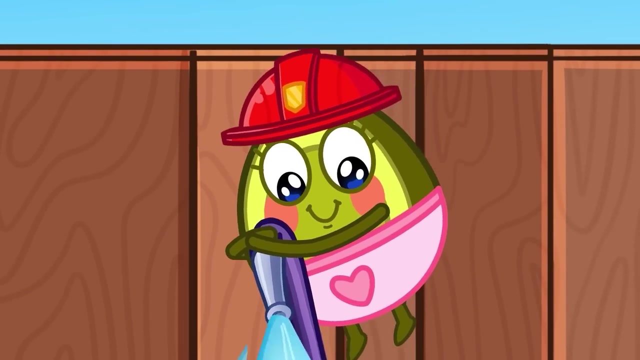 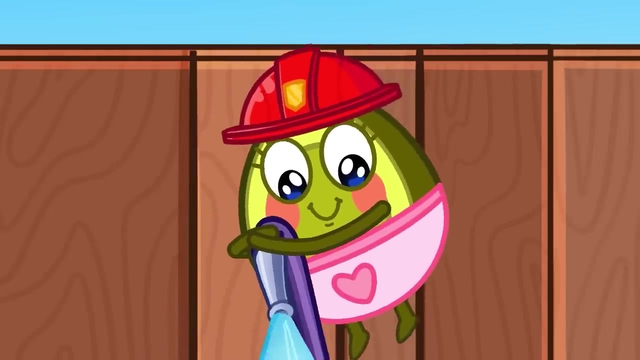 That's much better. Maybe she will become a firefighter. Okay, baby, Let's see if you can be a firefighter. Here's your fire hose to put out fires. Baby just wants to spray pit and penny Baby is too high. How can we get her down? 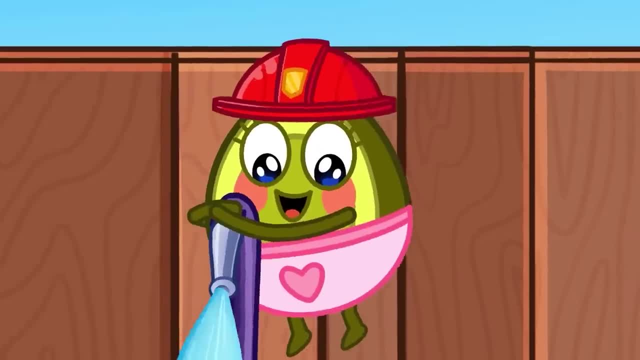 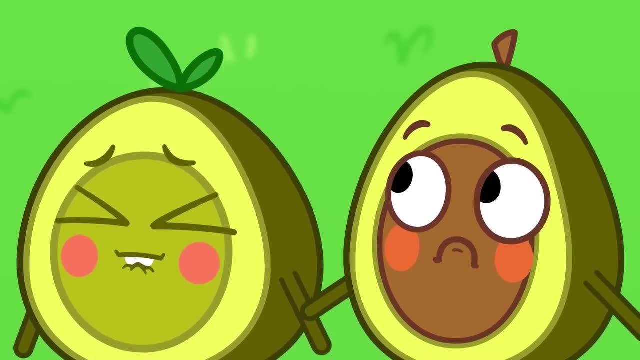 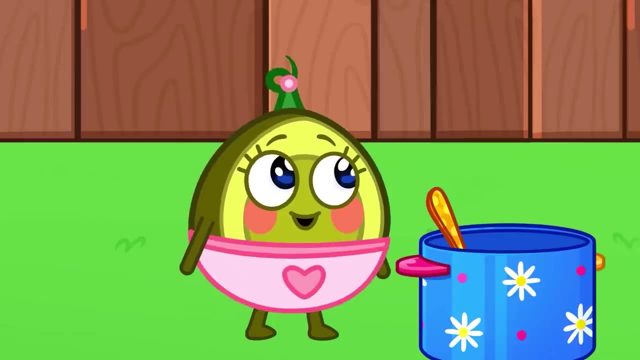 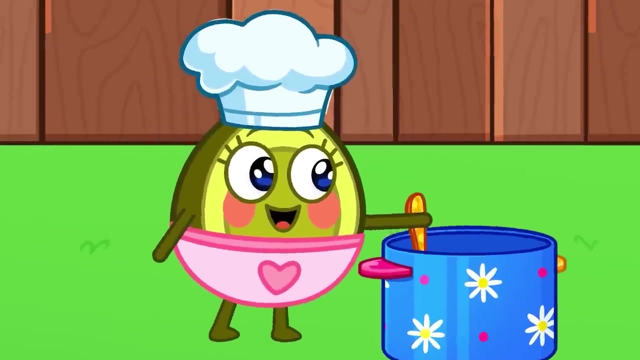 Pit will turn off the water And daddy will catch baby. We wanted to find a profession for the baby. Baby is too small to choose a profession. I don't know, daddy, Something tells me she might become a chef. Penny is playing doctor. 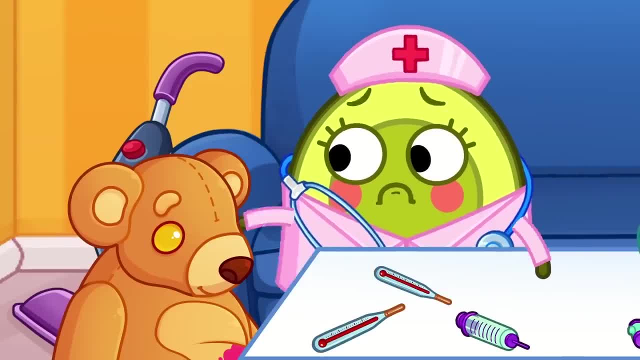 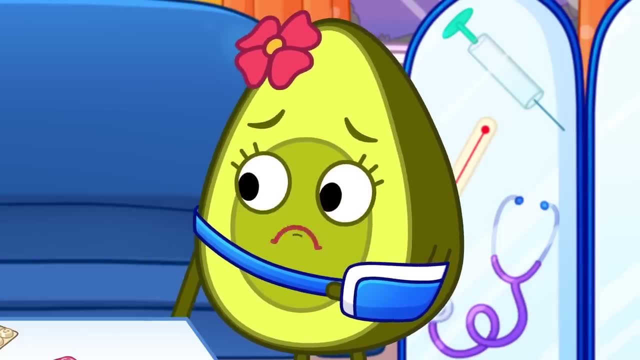 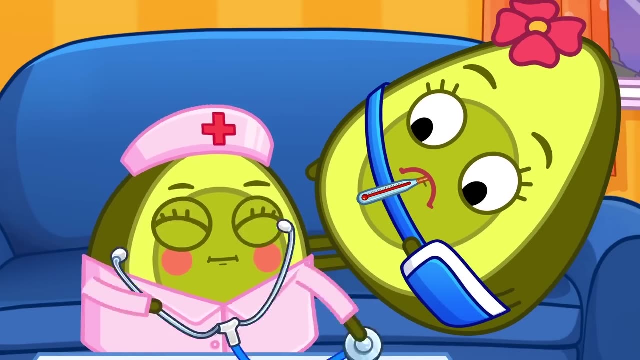 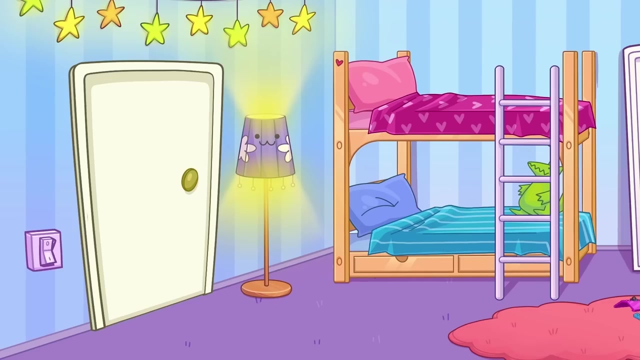 Teddy is feeling sick. Get better soon, Teddy. Doctor, my hand hurts, Help me. Doctor Penny tells mommy to lie down. Doctor Penny takes mommy's temperature. You'll need your medicine. bag Pit is pretending to be a builder. He is in a very tall crane. 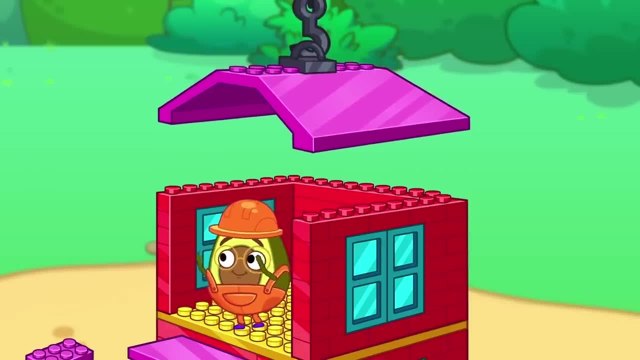 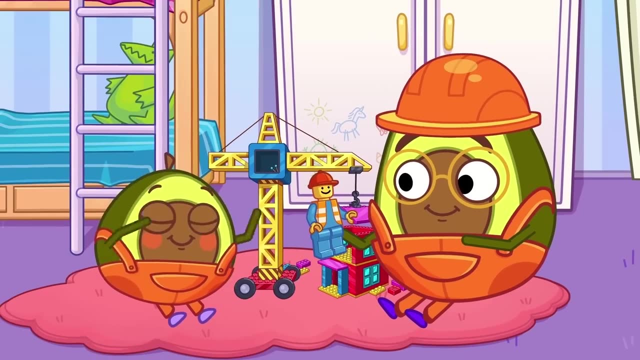 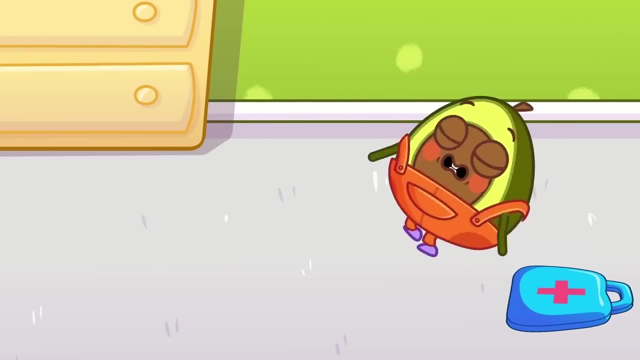 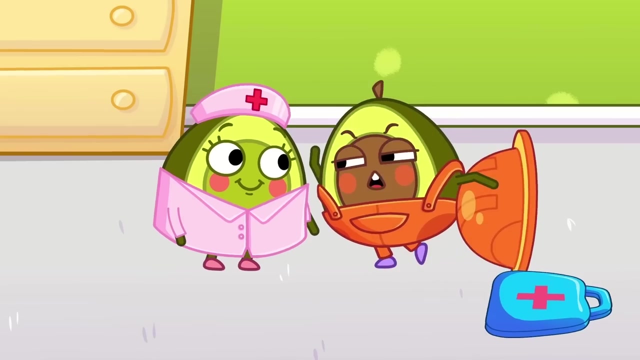 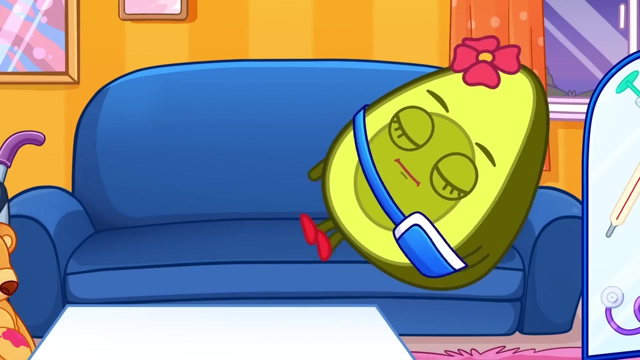 Daddy is helping Pit put the roof on the house. A builder must wear a hard hat. A hard hat keeps your head safe. Phew, Pit is okay. Pit has an idea. I wonder what's taking Penny so long? Wait, that's not Penny. 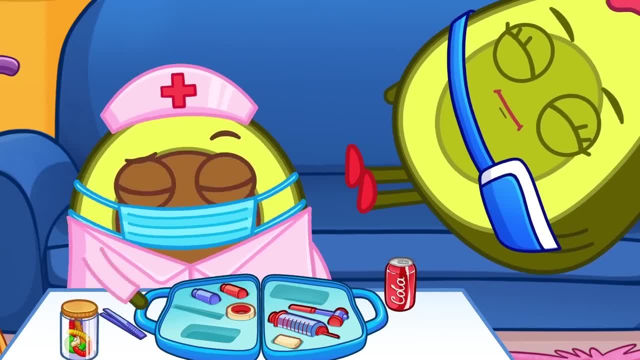 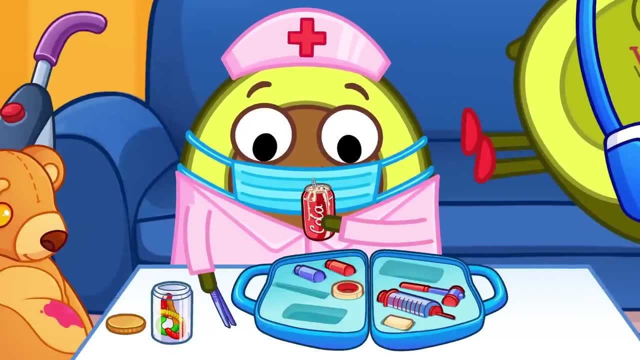 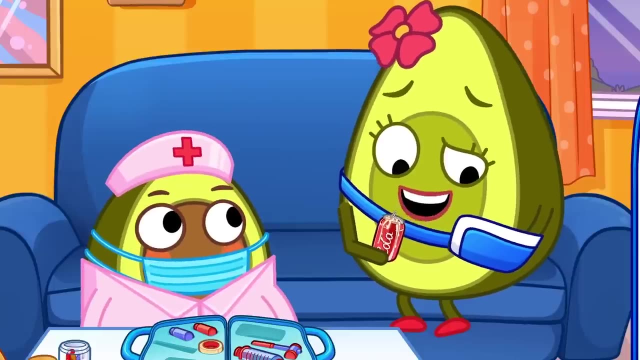 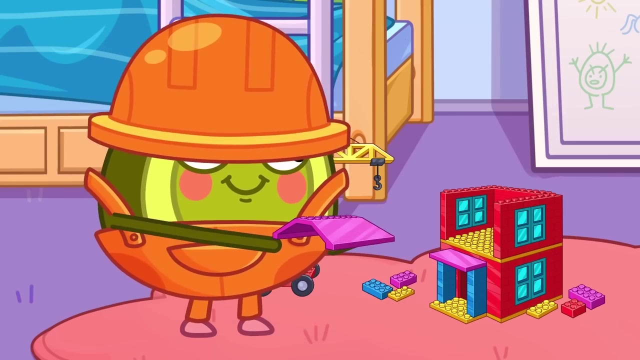 Penny. It's Pit. Pit and Penny are playing a prank. Pit is going to make mommy feel better. Pit gives mommy some medicine, Doctor, but my hand still hurts. Look, Penny is the builder. She is going to put the roof on the house. 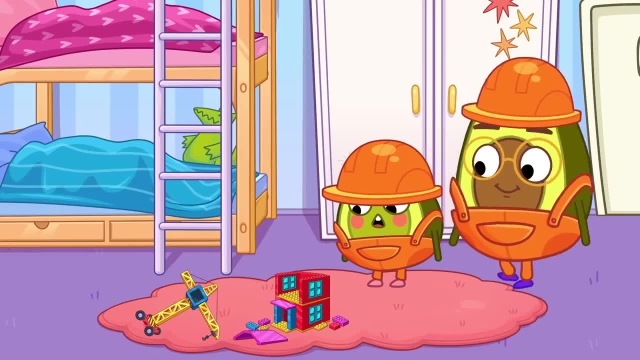 She has that money Nowもし я буду member of your family, she will let you go back. She will make mommy feel better. If she doesn't get the money, I'll have to make you go to the zoo. I don't want to be in the zoo. I want to stay here. You want to stay in the zoo. If she doesn't do anything, you will be coming back. You are going to be killed. I don't want to. This is a trap. Here you are, Penny. I will save you. Here you are, Penny, It's me. Here you are, Penny, It's me. I don't want to be a coward. I don't want to be a coward, I want to make you go home. 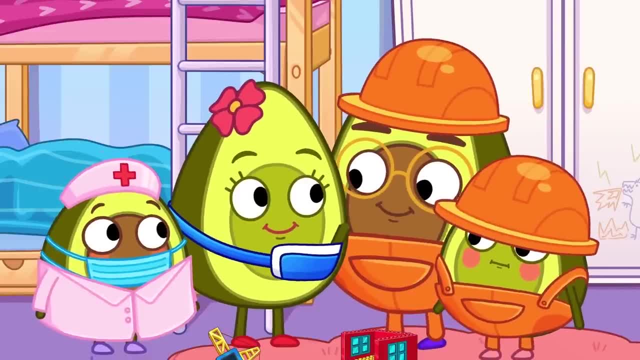 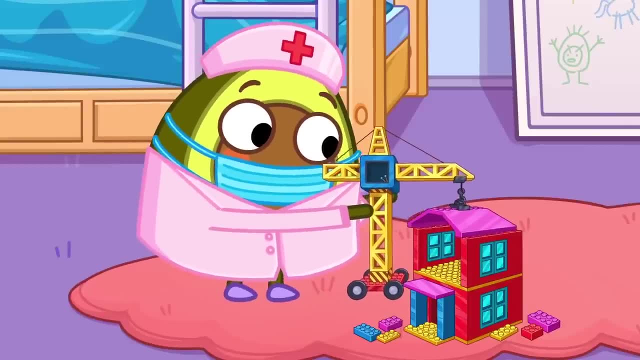 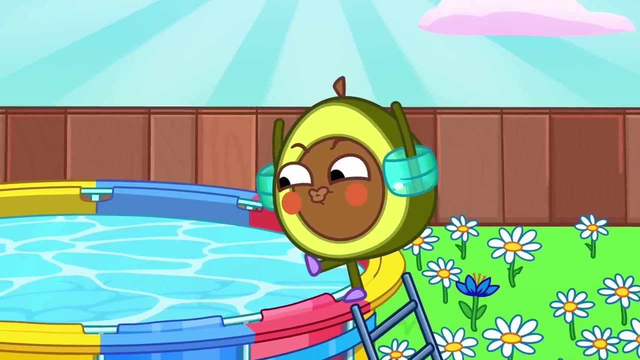 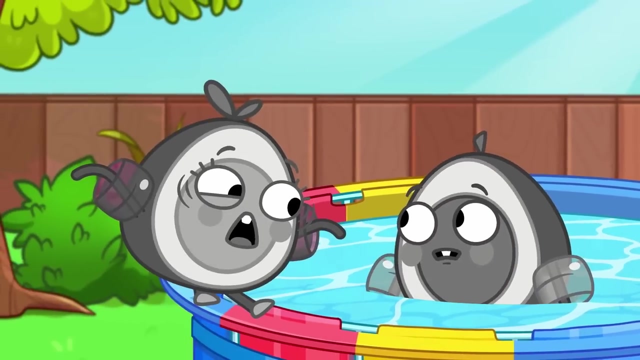 I don't want to be a coward, So a doctor can do a builder's job. Penny fixes Mommy's hand. Well done, Pit. Pit and Penny are playing in the pool. Animal. Oh no, Pete, Our collars are gone. 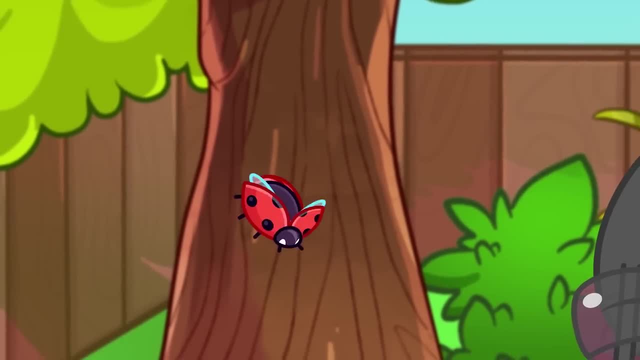 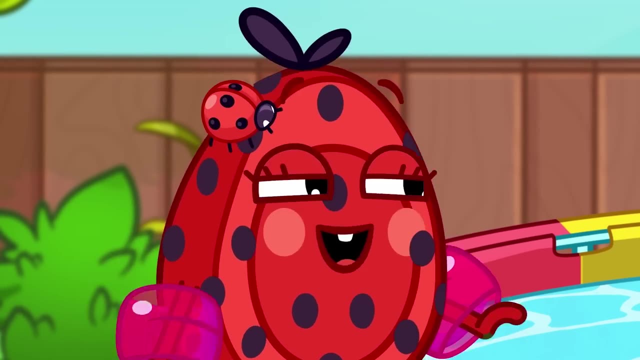 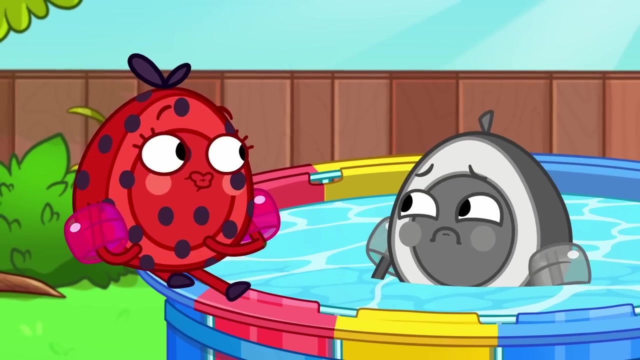 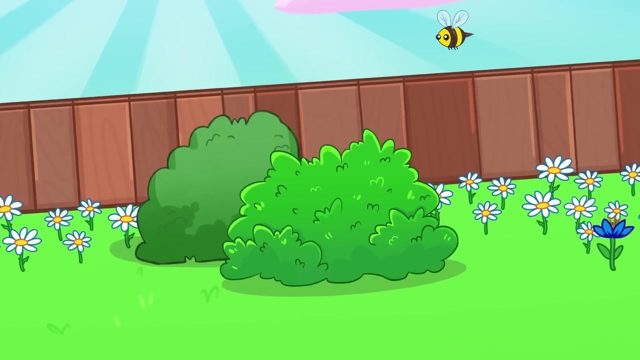 How will they get their collars back? Penny, you look different. I'm a ladybug now. Cool, I want to find a collar too. Look, Pit, it's a black and yellow bee. There's a chipmunk on your head. 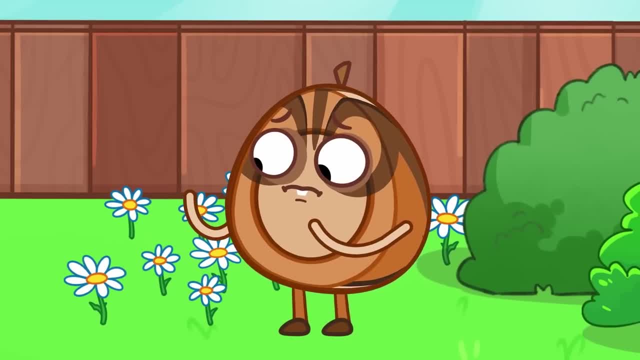 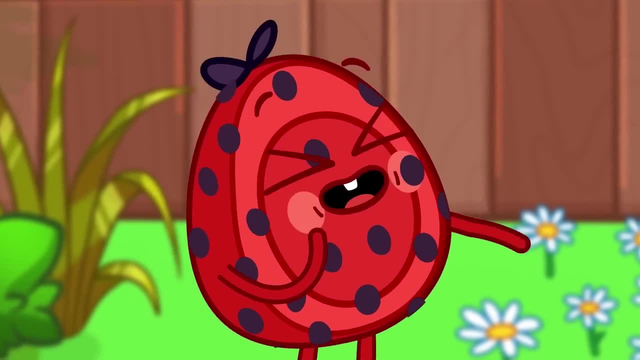 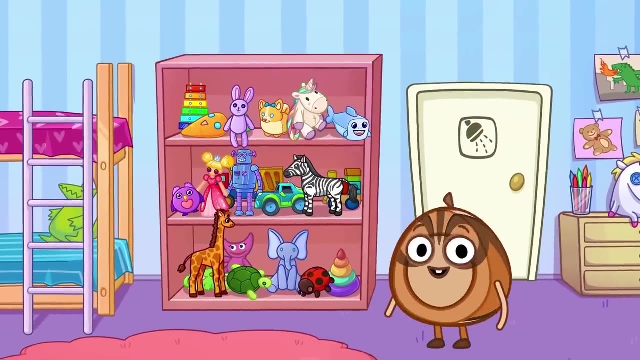 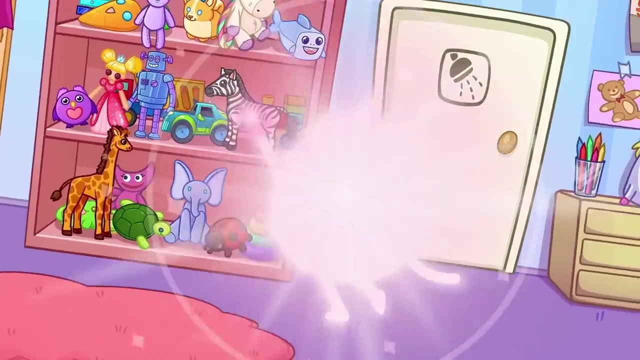 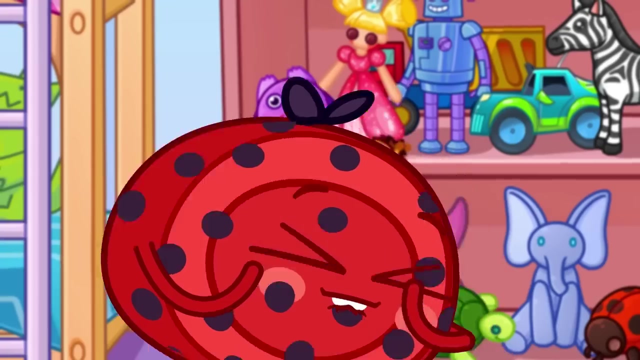 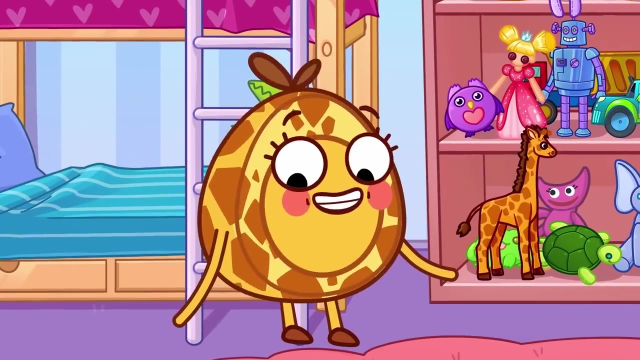 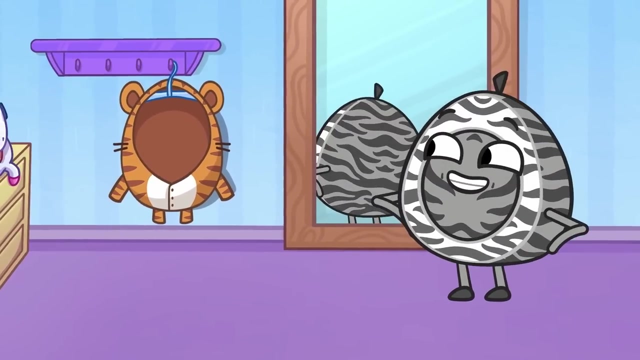 Oh no, Pit's collars changed. Oh no, Pit wants different collars. Zebras are black and white, And so is Pit. Penny wants to try. She picked the orange and brown draft. It's even better Now. Pit wants to be a tiger. 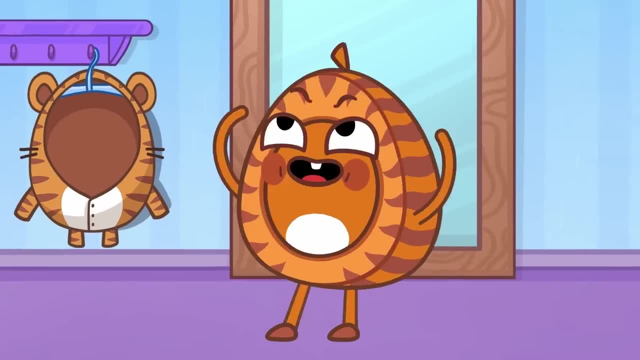 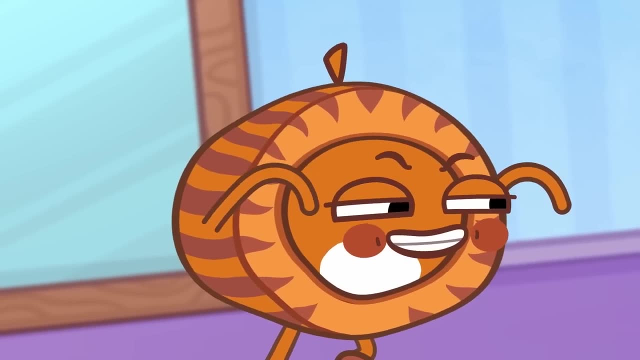 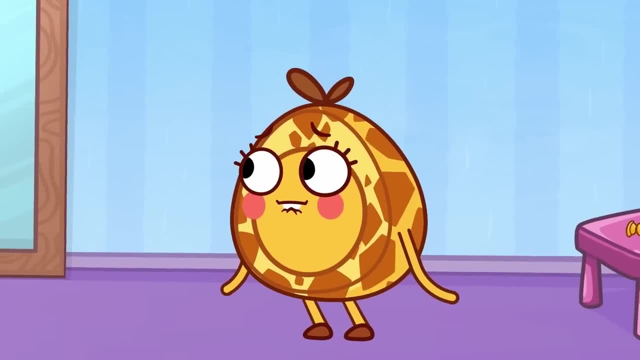 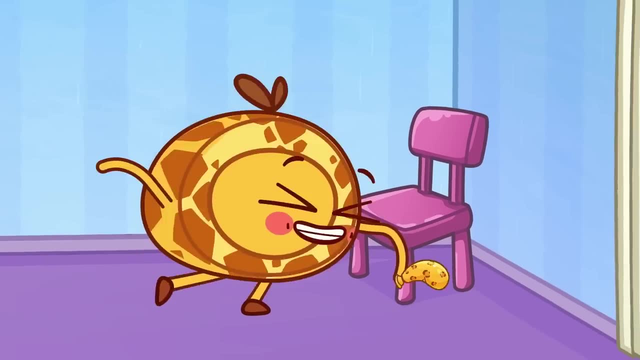 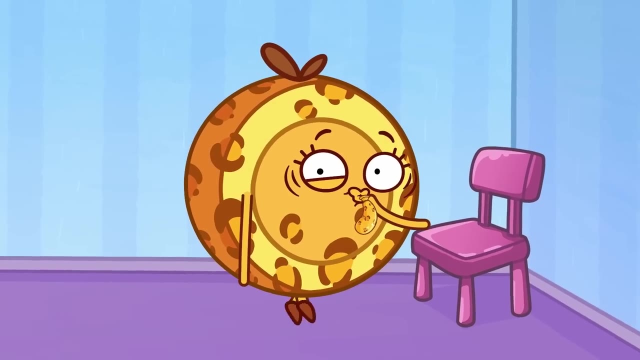 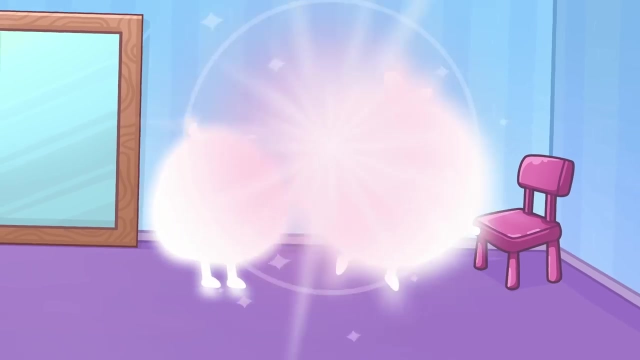 No, No, No. Now what will Penny choose? I'll be a predator too. She wants to be a leopard. Oh no, Penny needs help. Penny lost all her color. No, No, It's because she is too beach happy. 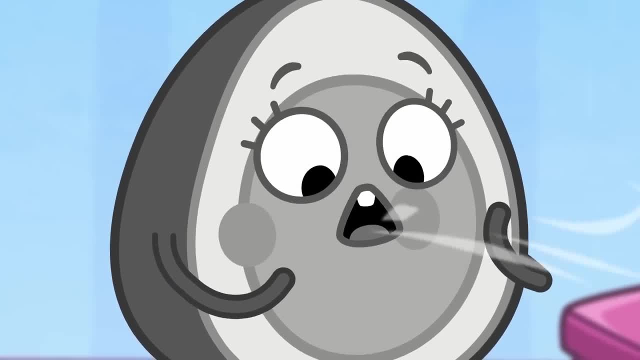 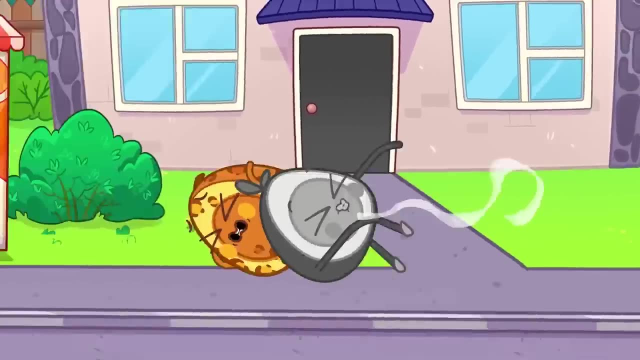 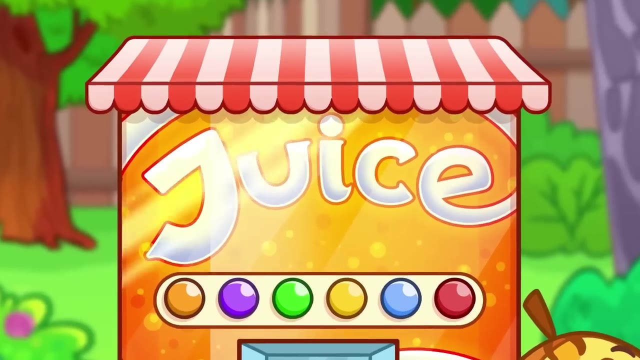 Ouch, She almost landed on the water. Will she please pull off an orange queef fly? I was wrong. Moreover, she has her pants all wet. Look, kids, it's a colorful juice machine. Wow, Pit picked a red juice. 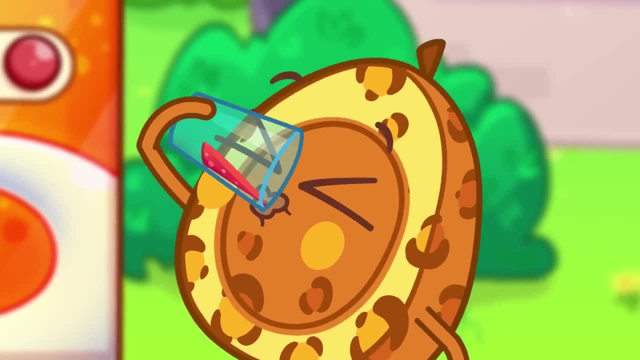 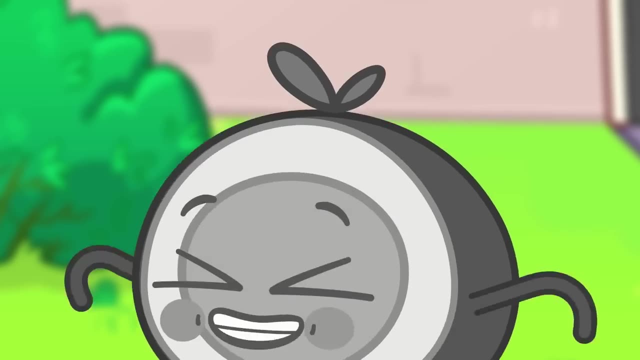 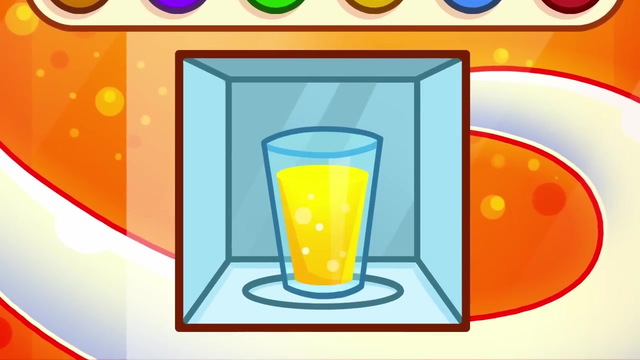 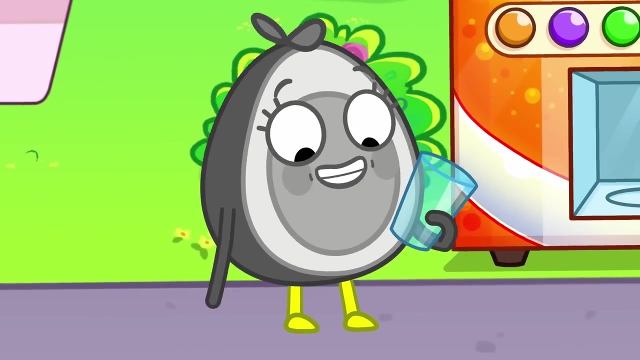 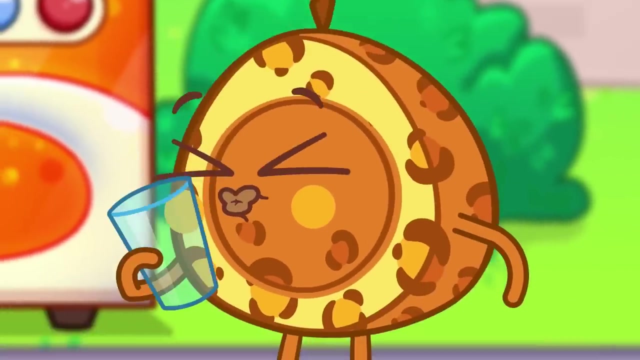 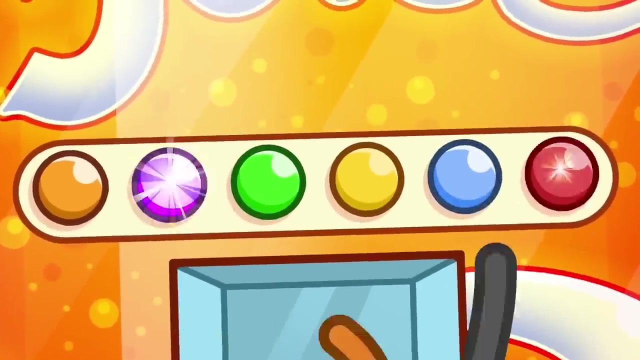 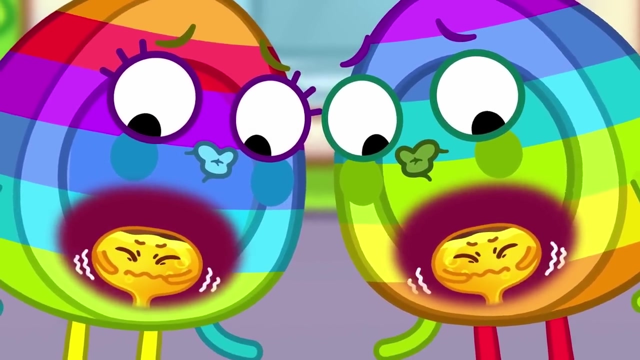 いる 내일. Yes, His legs are red, So cool. What will Penny pick? She picked yellow. Yummy, yummy. And her legs are yellow. They want to try all the colors. They've become rainbows, Uh-oh, They need the potty. 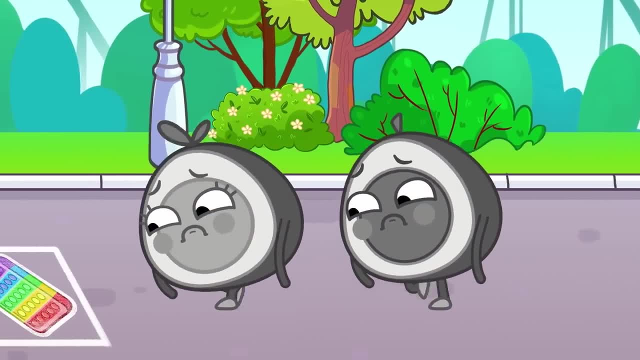 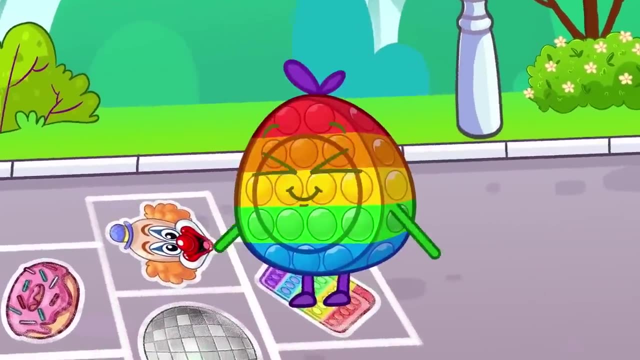 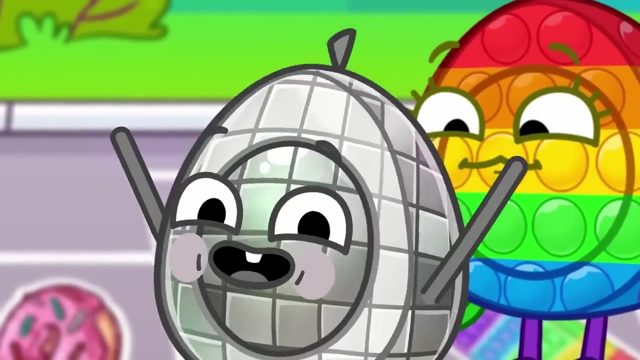 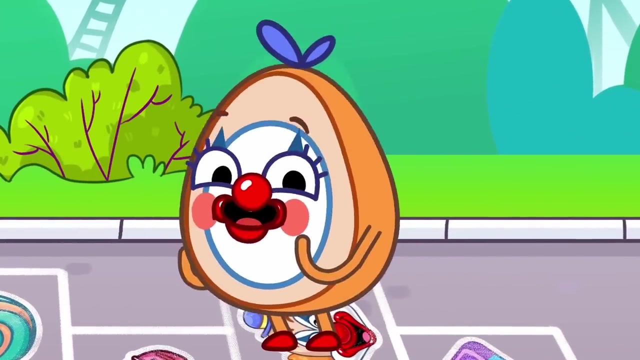 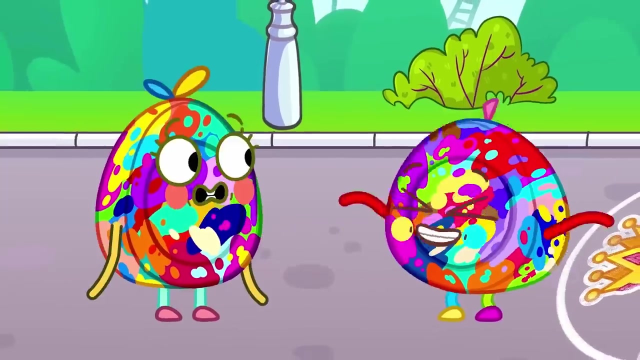 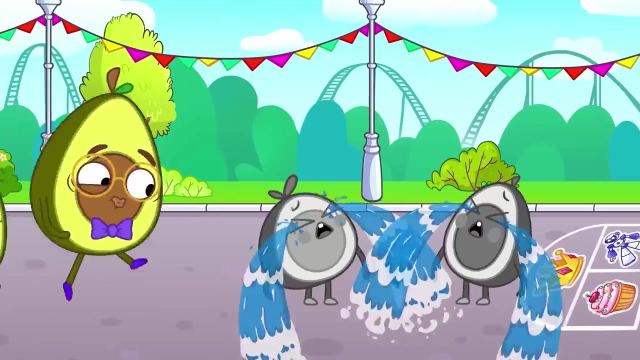 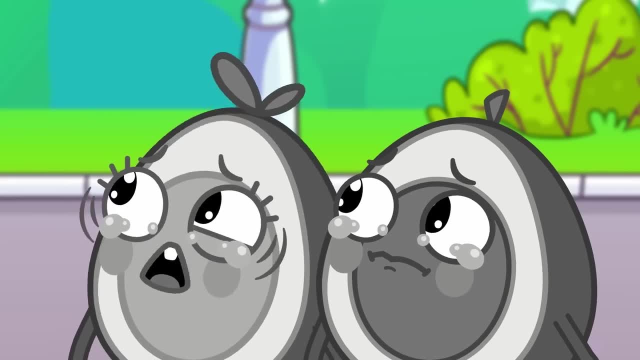 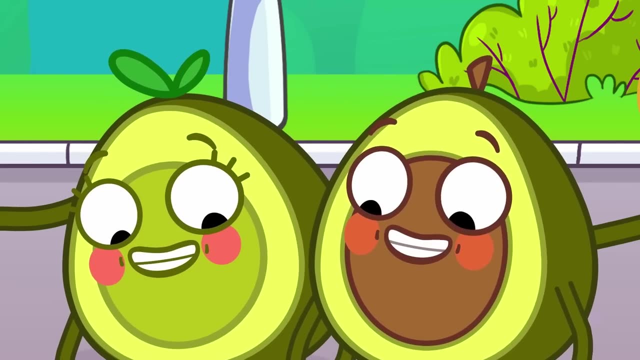 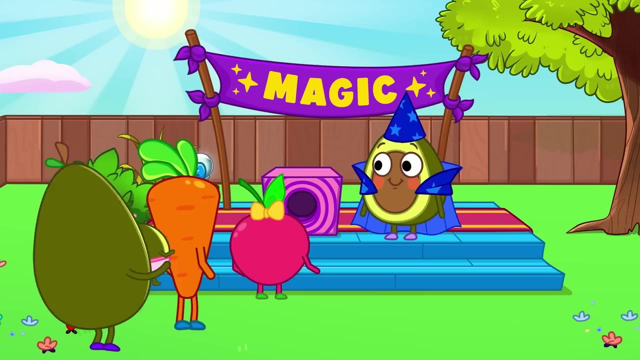 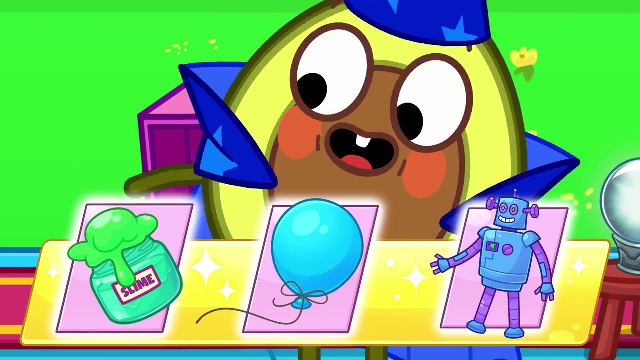 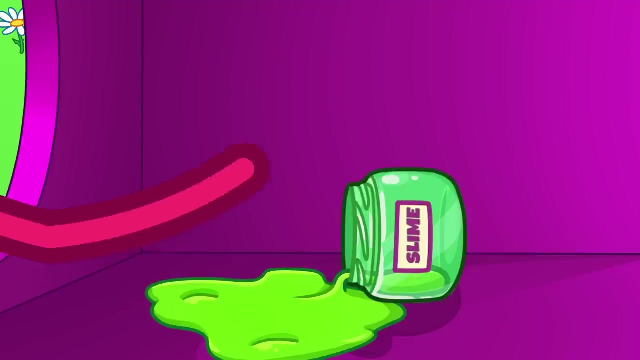 What's happened? We can get our colors back. Well, that we can fix. Mommy and Daddy saved the day. Kit has a special mystery box. What will he hide inside? Guess what's in the box. What was it? Cherry? 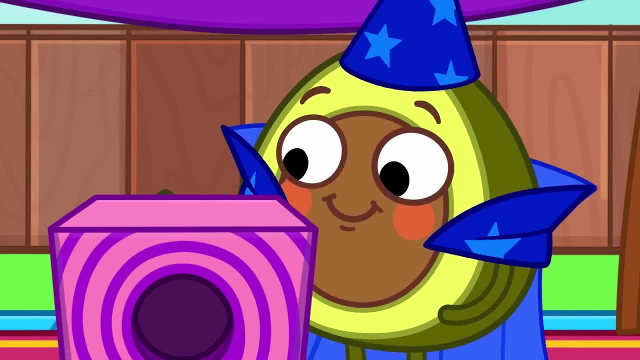 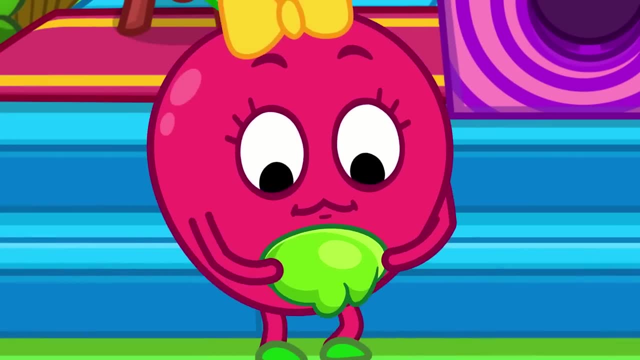 It's a talus fish. Wrong. It was play slime, Play slime. This is for you. It was a snake, You're so sweet, You're so sweet. It's a plant. It goes inside my clothes, Oh, Oh. 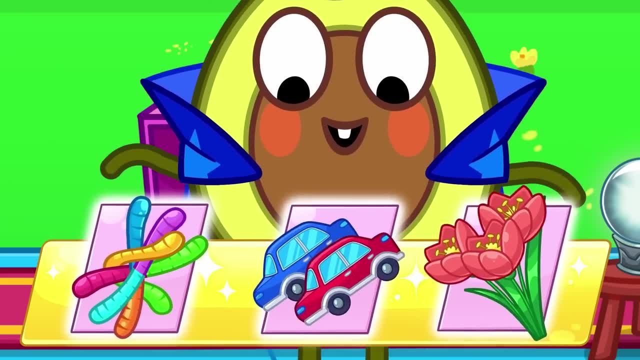 Oh, Oh, Oh Oh. What should Pit hide for Carrot? We're all welcome here. We'll find out about it later And we'll see you later. We're all ready. We're ready to go, We're ready to go. 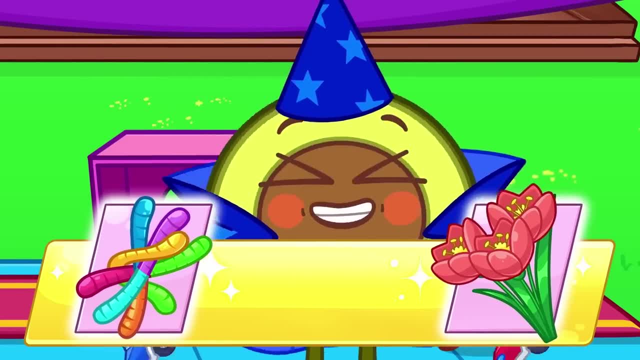 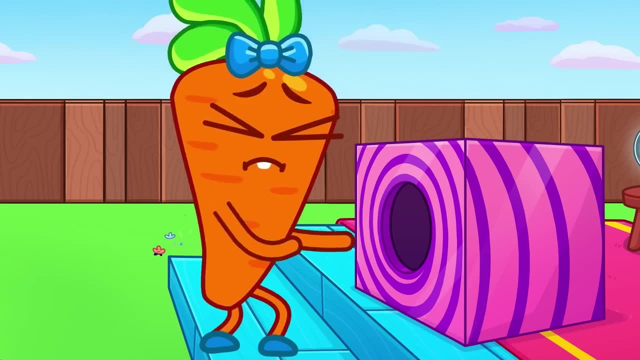 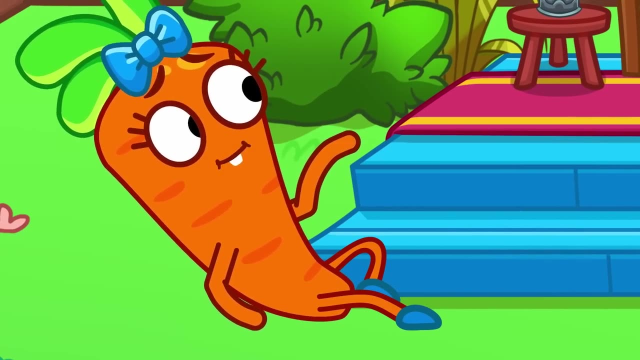 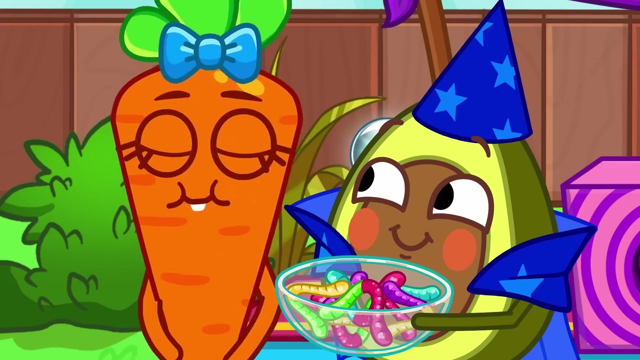 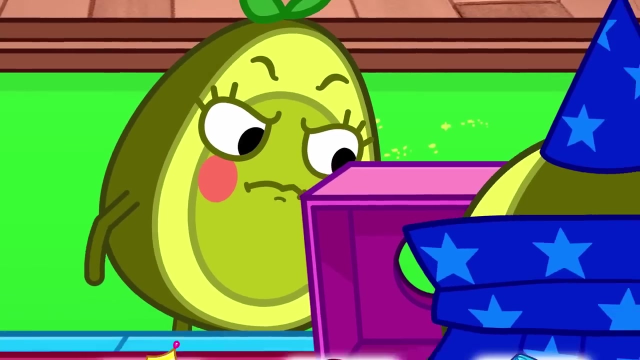 Cars are boring. Guess what's in the box. Guess what's in the box. Guess what's in the box. It's worms. Almost They're candy worms. I won't be scared. What will Pit pick Shh? Don't tell Penny. 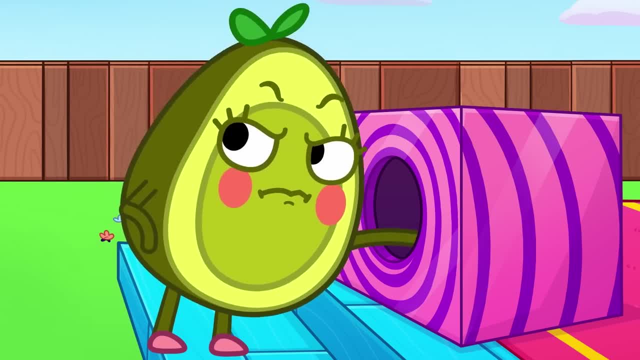 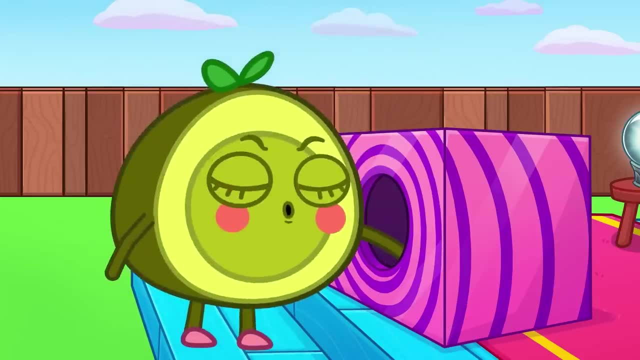 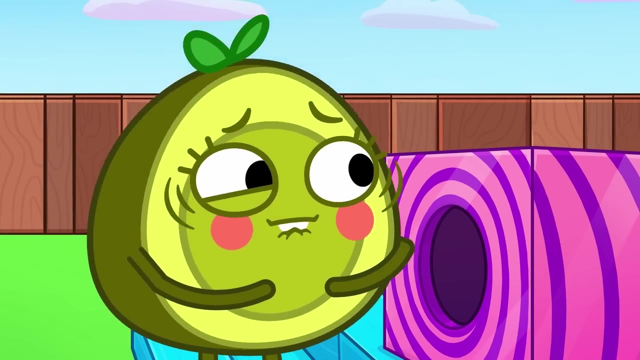 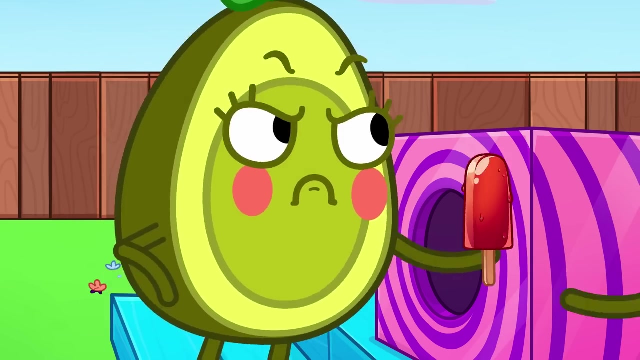 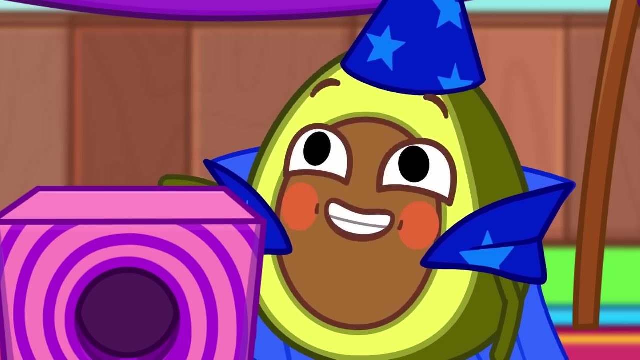 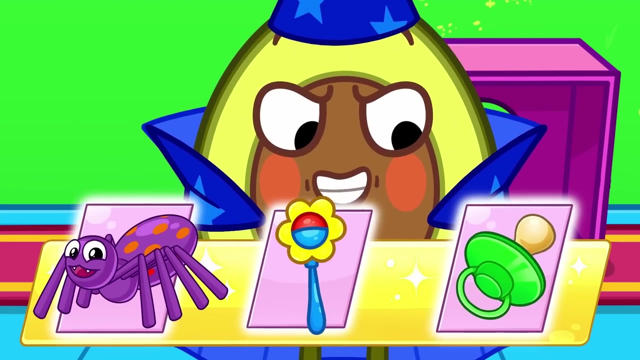 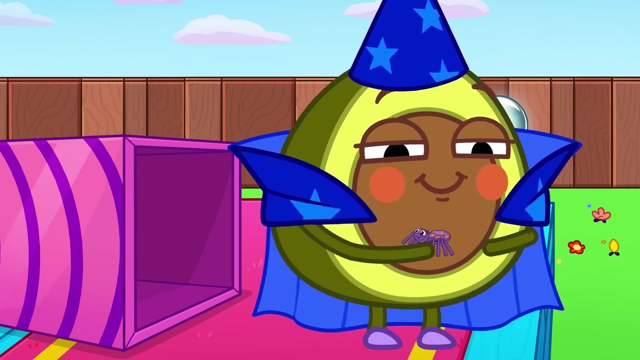 Well, come on, Do it. What a cold surprise. Is it a monster's tongue? It's not fair. It's a popsicle. Can I guess what's in the box Now? what will Pit pick? Okay, Daddy, It's your turn. 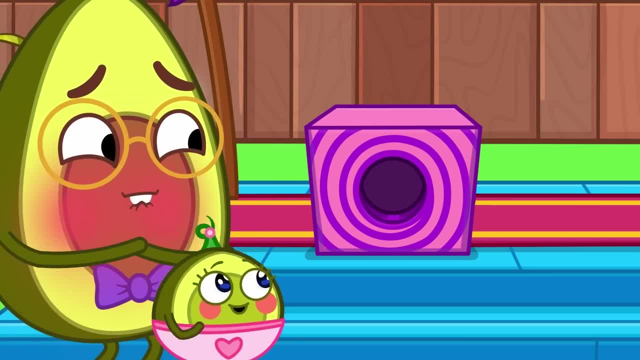 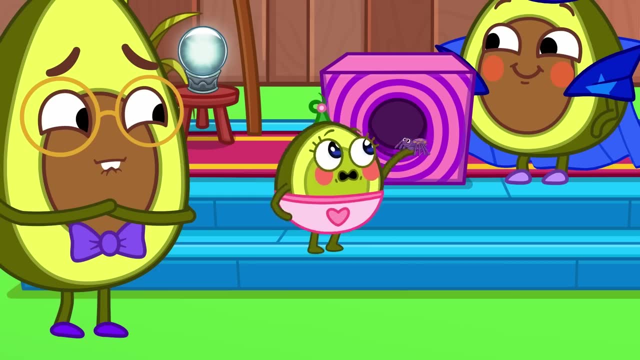 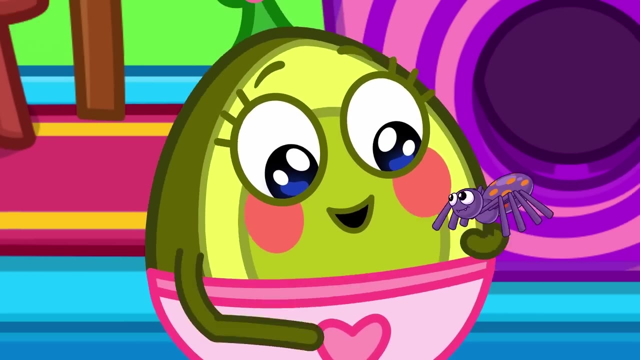 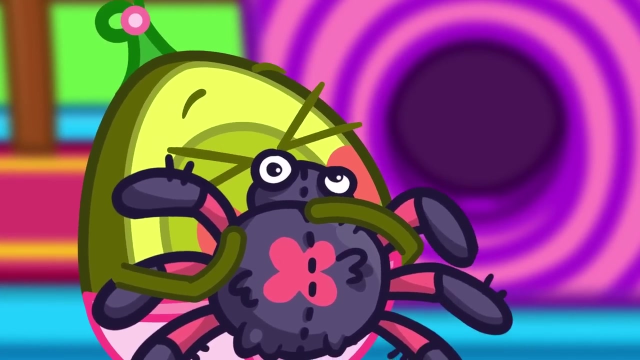 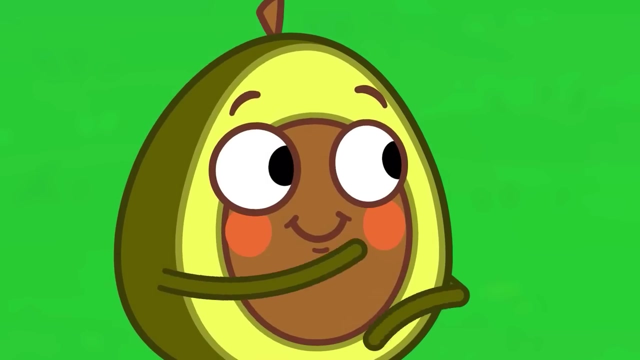 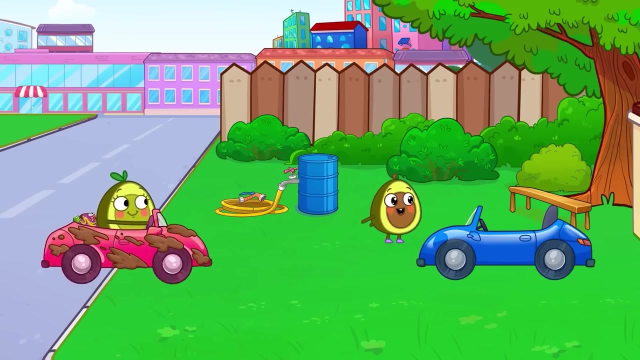 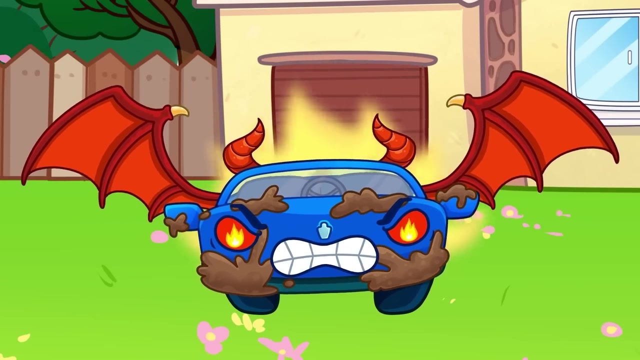 Daddy is afraid. Oh, A spider. Daddy doesn't like spiders. And we have a winner. Well done. baby Pit is washing his car today And now it's clean and shiny. Now it's covered in mud. Hurry Pit, Being dirty makes Blue Car angry. 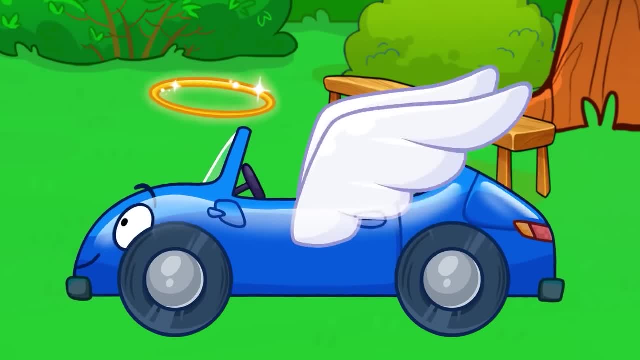 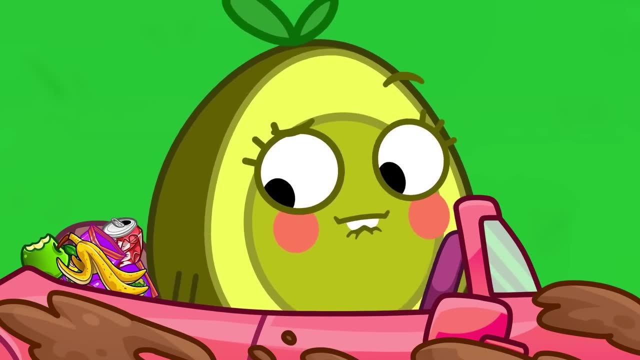 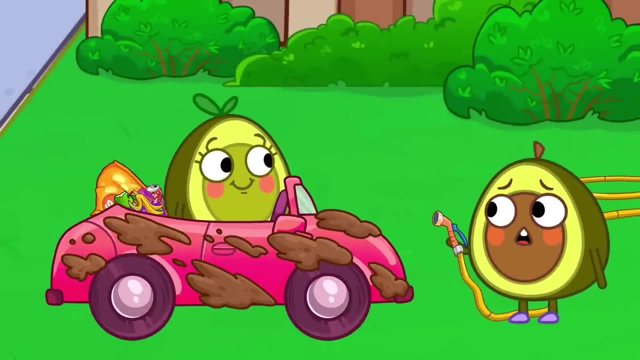 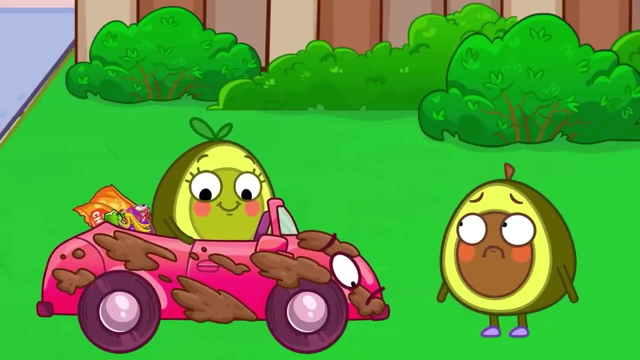 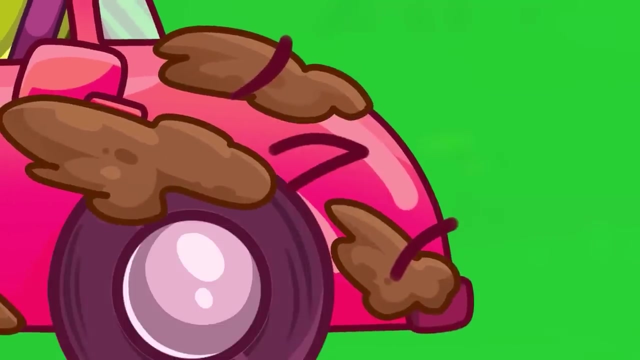 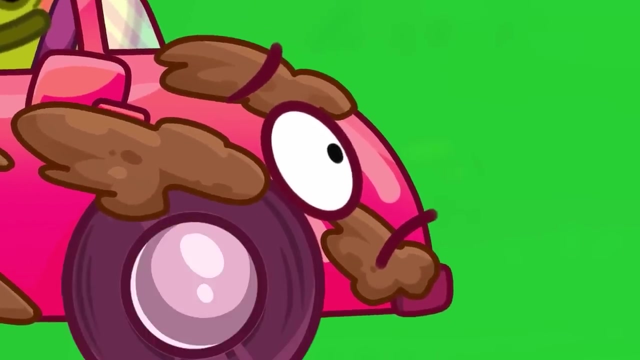 Much better. Now let's clean Penny's car. What's that smell? Oh, Oh, What is that smell? Oh, But Penny, your car is a mess. Be careful, Penny. Pink car is sad. That will make pink car mad. 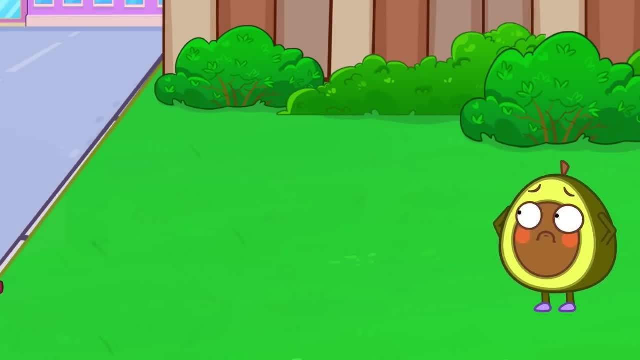 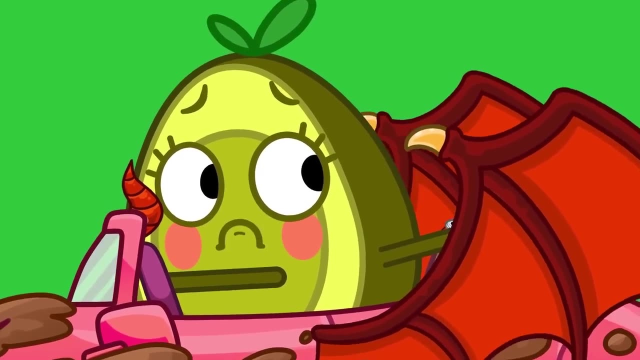 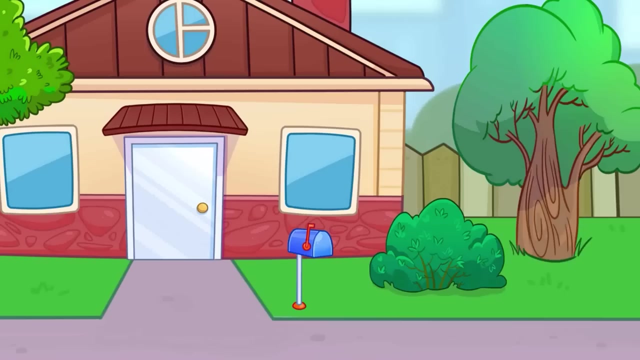 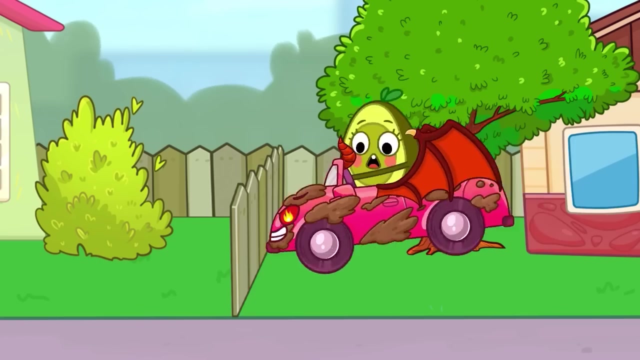 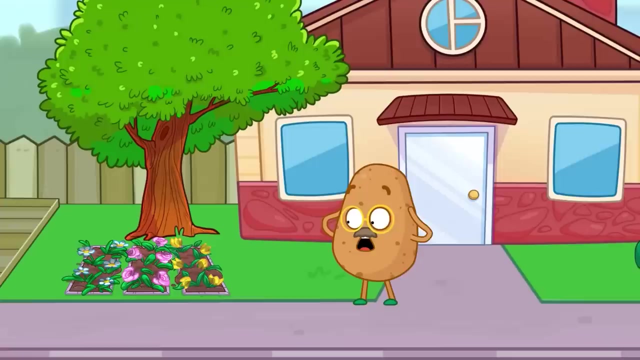 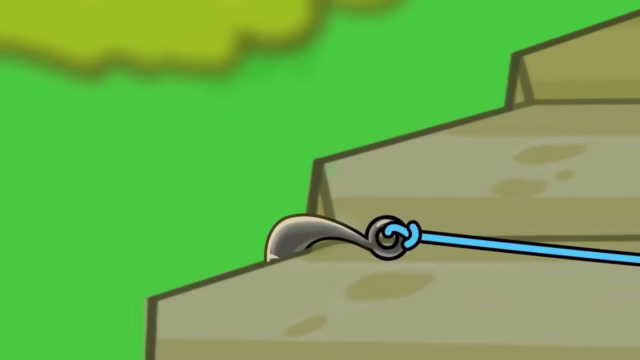 Oh no, Penny is stuck. Hurry Pit, Penny needs you. Pete, help me. Oh no, The mailbox. Oh no, The flowers. Oh no, The fence. Mr Potato needs your help. Pit, Well done. 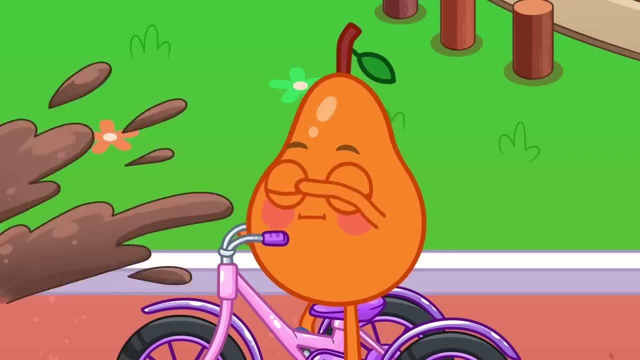 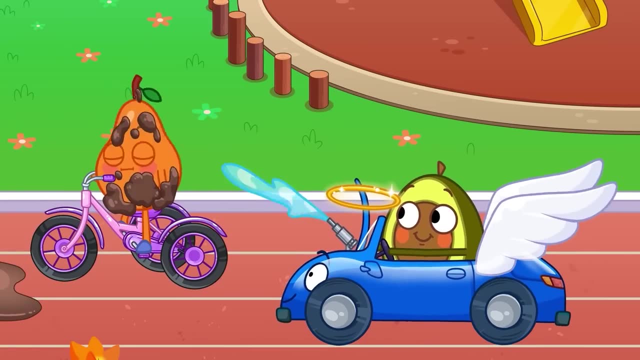 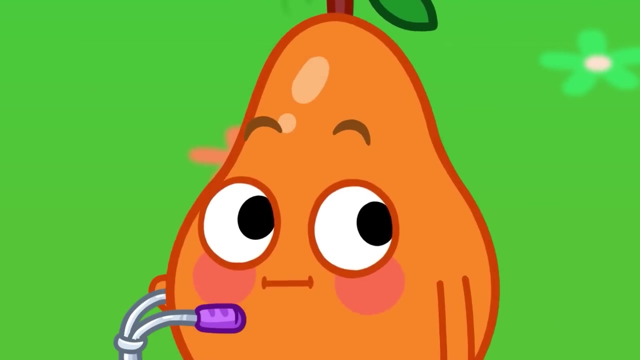 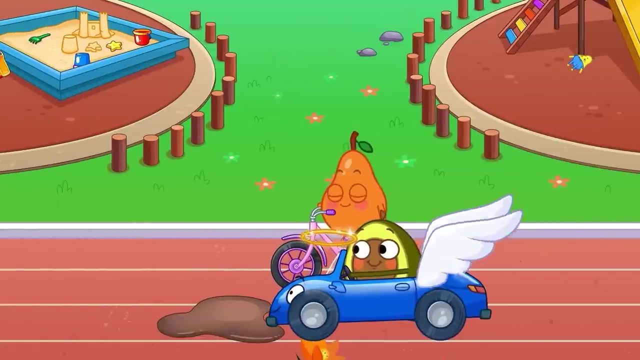 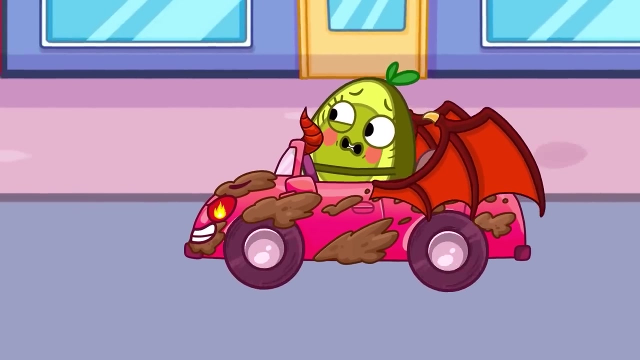 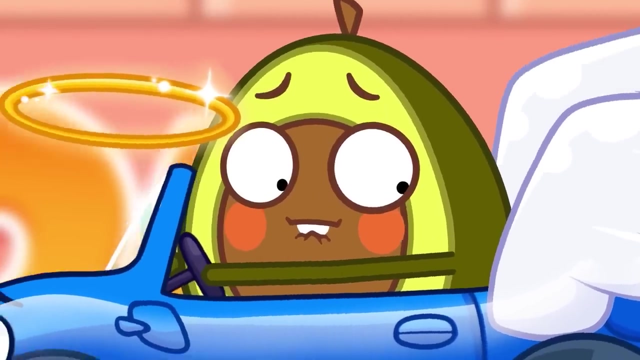 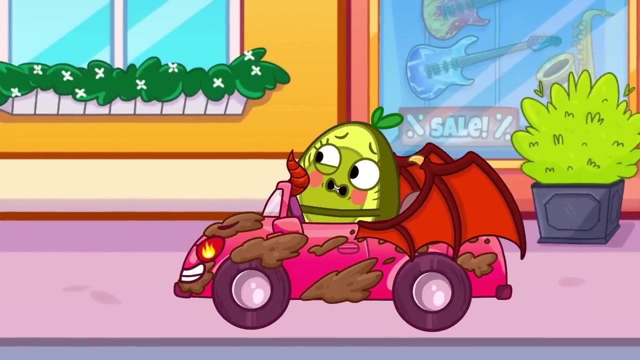 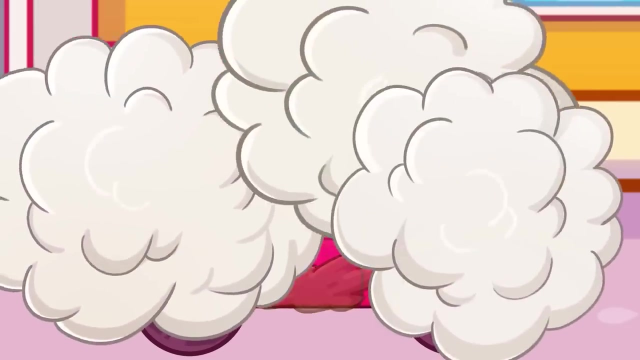 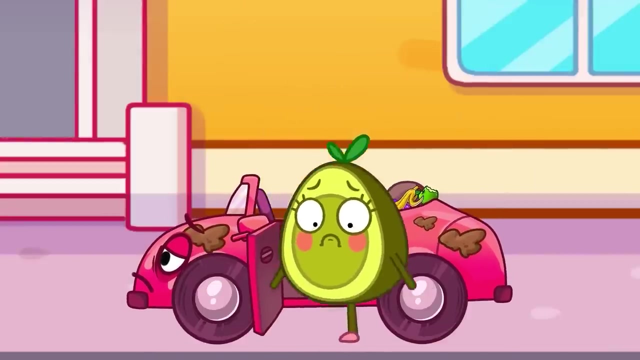 There's a puddle in Perry's way. Poor Perry. Maybe Pit can help. First a wash, Then a wipe, Now up and over the puddle. Now, Pizzy, tell Blue car, use your wings. It's safe to come out, Penny. 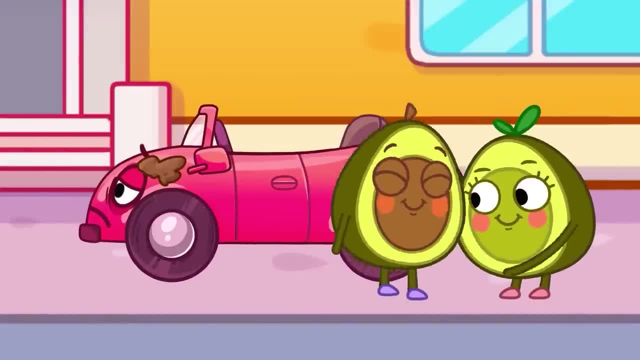 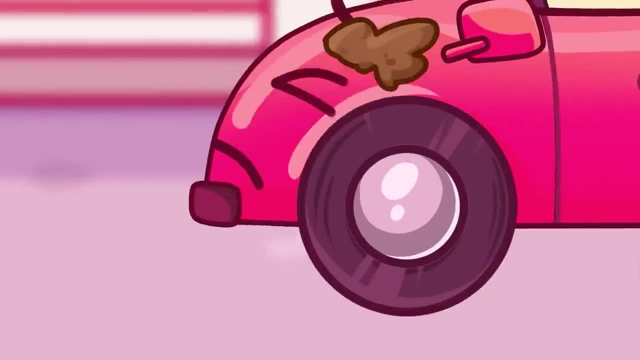 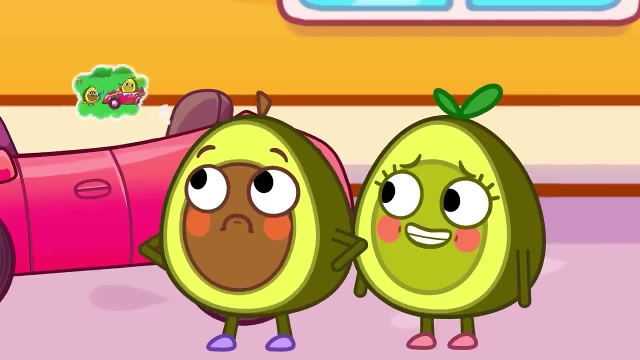 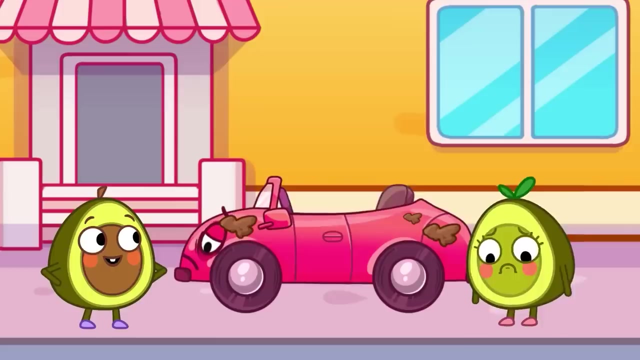 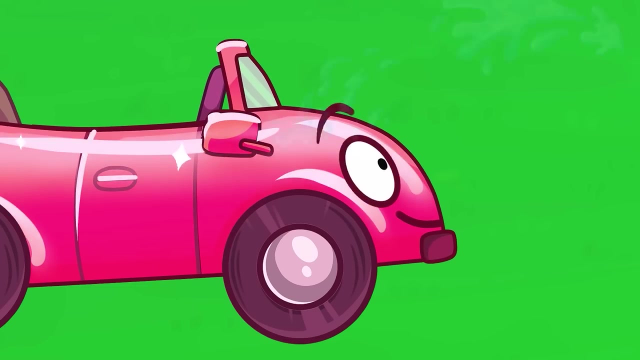 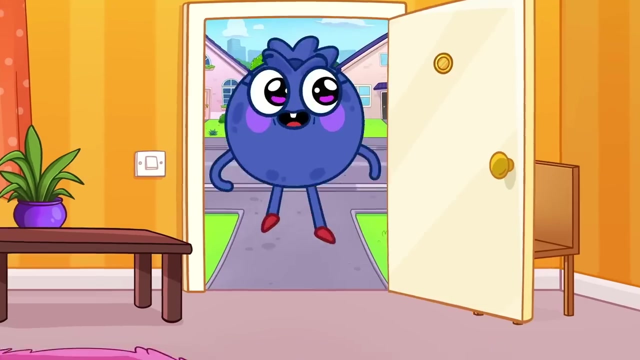 Oh, it's me, But pink car is still sad. Oh, What's wrong pink car? Penny treated me really badly. Treat your car like your best friend Penny. Pink car is much happier now. Good job, kids. Blueberry has come to visit. 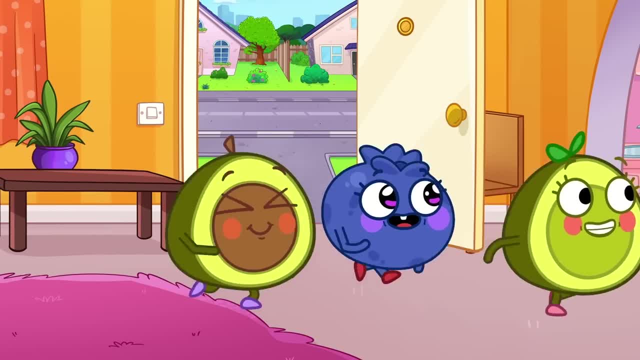 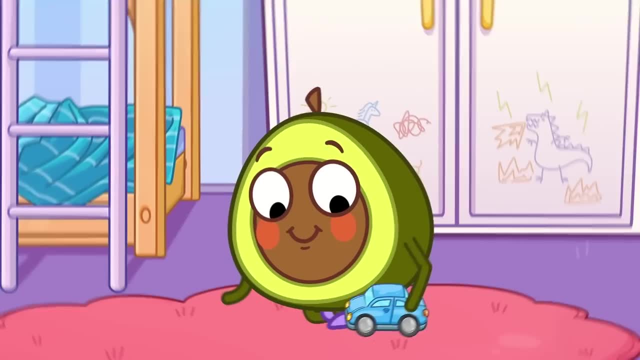 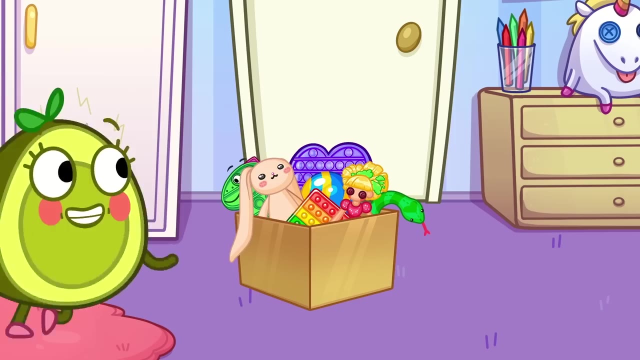 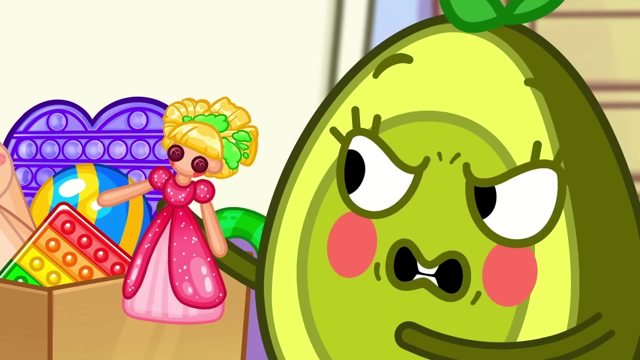 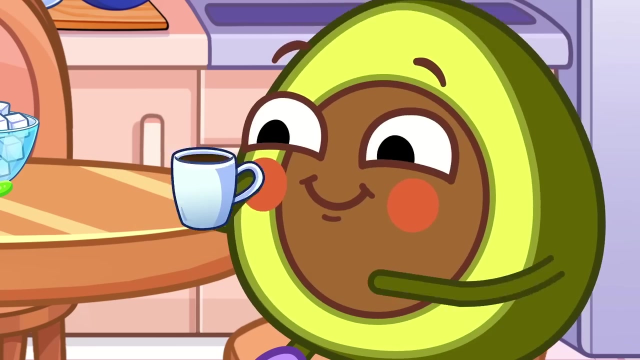 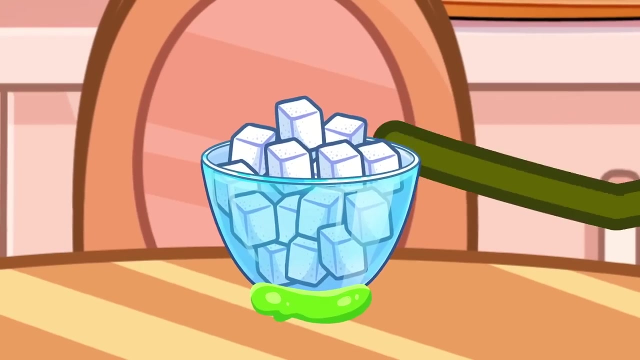 Come on, Let's play. Why is Pit's car so sticky? Someone put a booger on it And there are some on Penny's doll. I love these boogers. I like my tea sweeter. Even the sugar bowl is sticky. 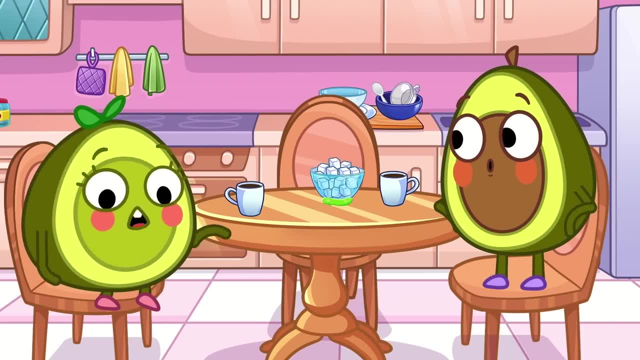 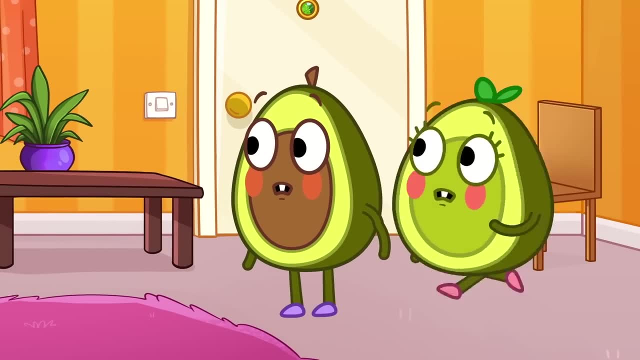 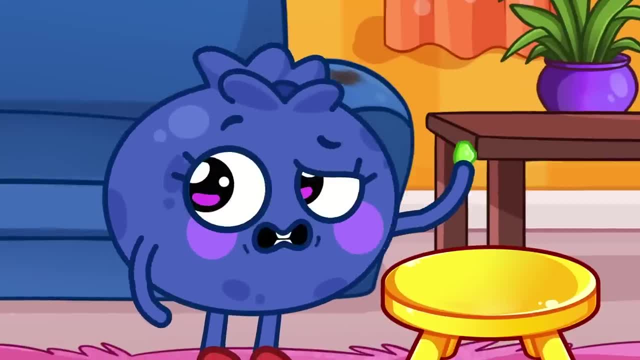 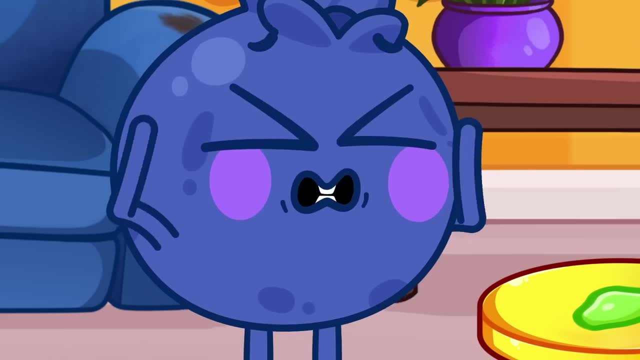 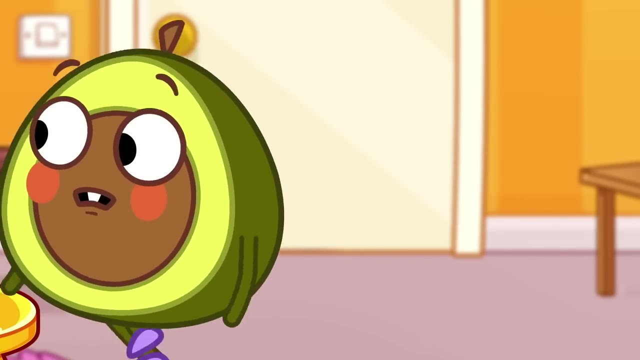 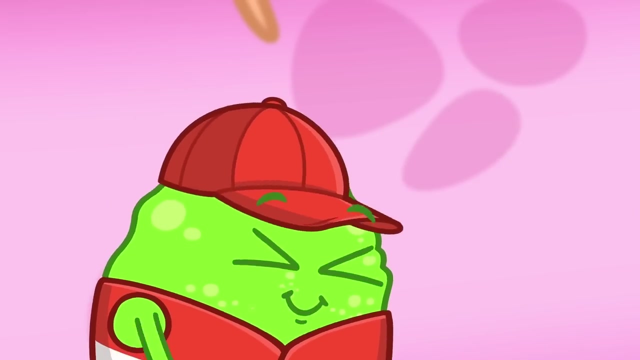 Look, Look, Look. The problem is. The problem is Blueberry. That's not nice Pit, You shouldn't laugh. There is nothing to worry about. Why is that? Penny Boogers collect dust in our nose so that we can breathe clean air. 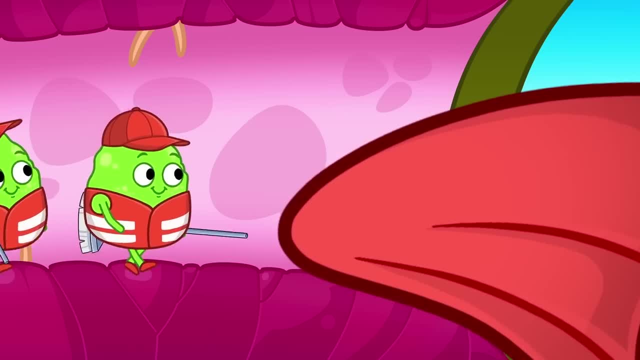 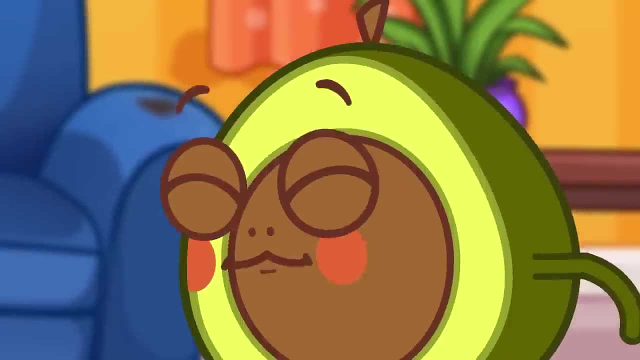 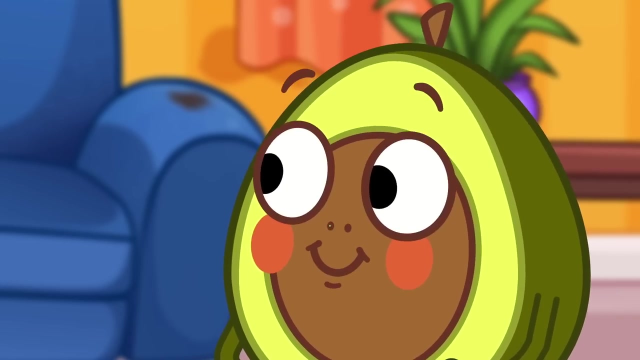 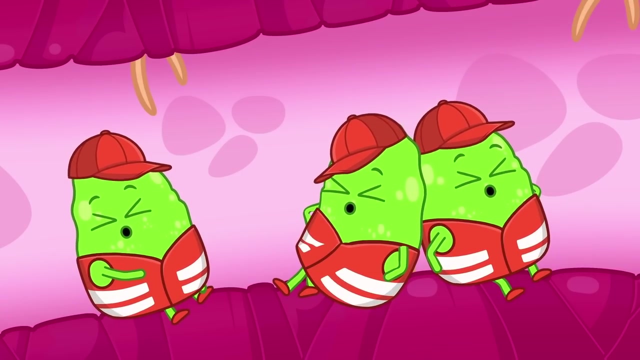 The best tool for them is a hanky. Always blow your boogers into a hanky or tissue. See, Pit has boogers too. Look, Pit's boogers got wet. That's because they guard our health. Look, Germs are coming in. 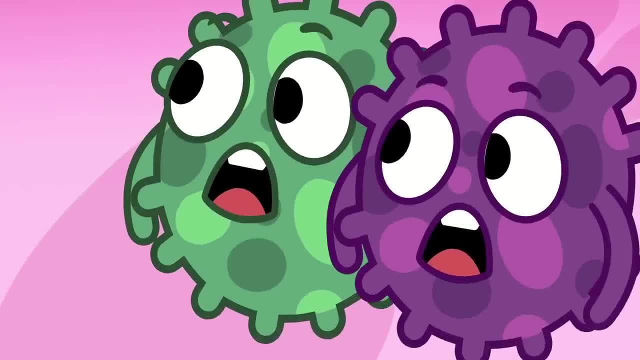 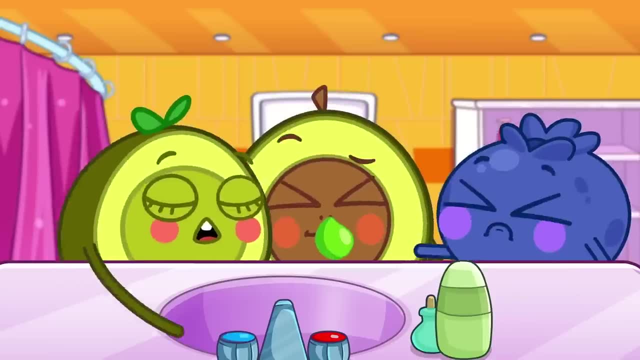 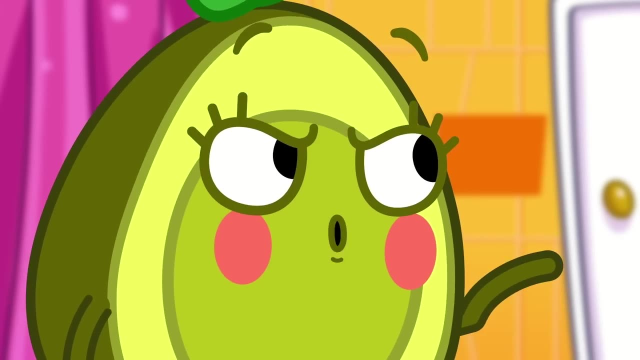 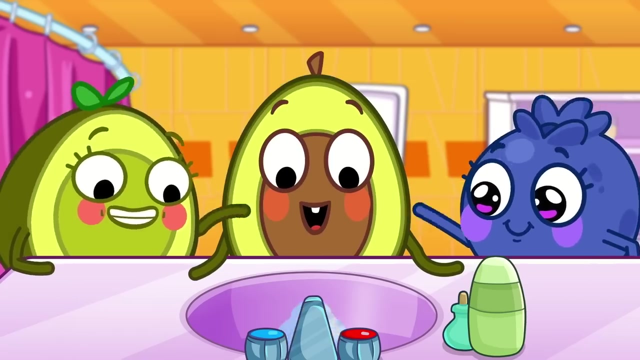 A rotty nose Keeps germs from entering Your body. Bless you, Pit. Now what should Pit do? You need to blow your nose. Blow harder Now the germs are gone. Hey, I have a surprise for you. 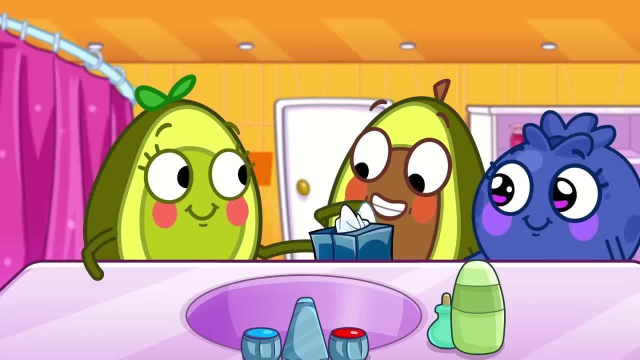 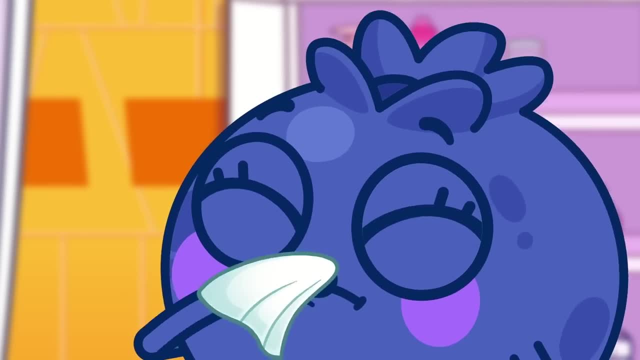 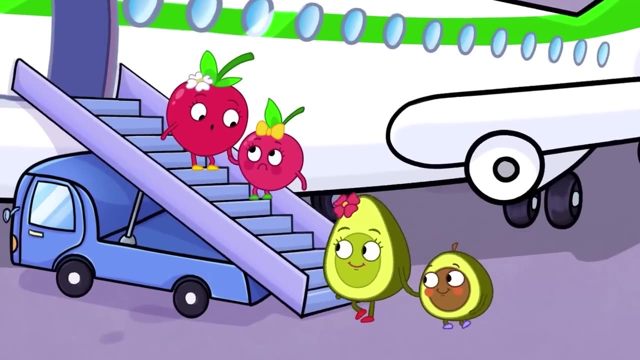 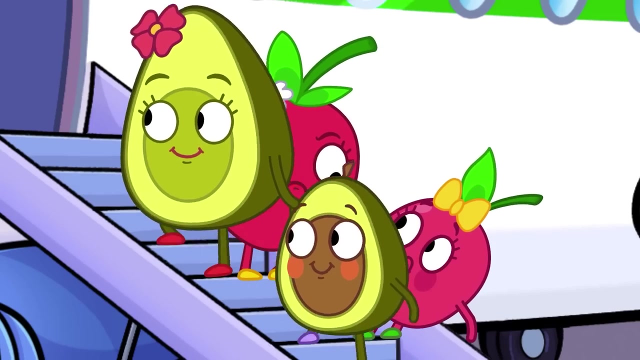 It's a box of tissue. Don't keep it. You have to keep it to yourself. See, That's where boogers belong. It's time for a plane ride. What's wrong, Cherry? I'm afraid of flying Pit. can you help, Cherry? 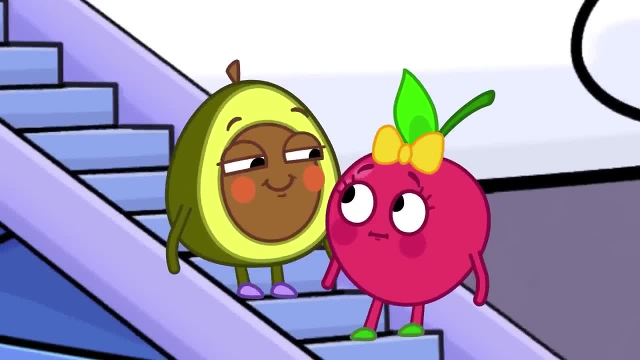 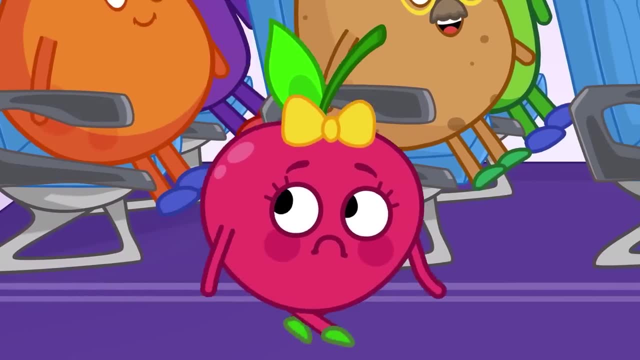 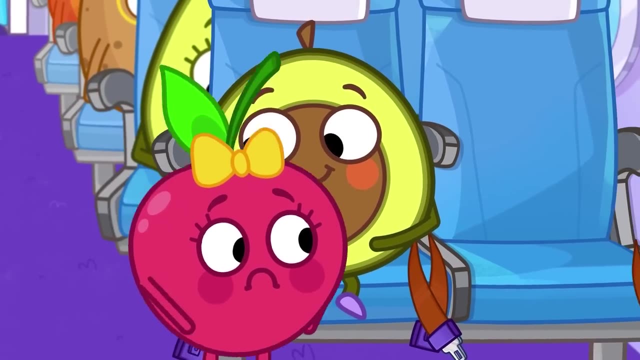 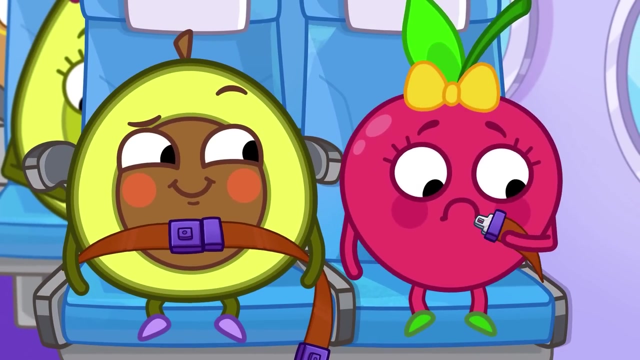 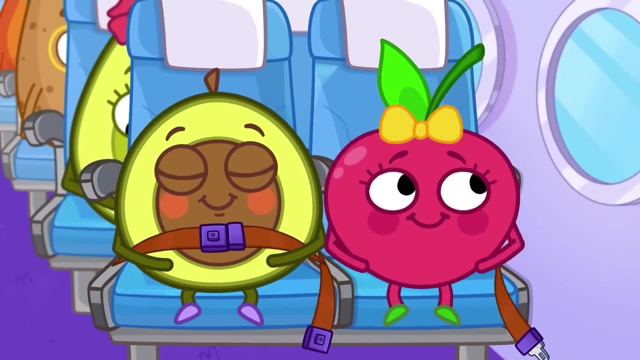 Pit, I will help you, It's not scary. Well, Cherry Hit, and Cherry can sit here First. you must always fasten your seatbelt, But Cherry doesn't want to. Without your seatbelt you might hurt yourself. 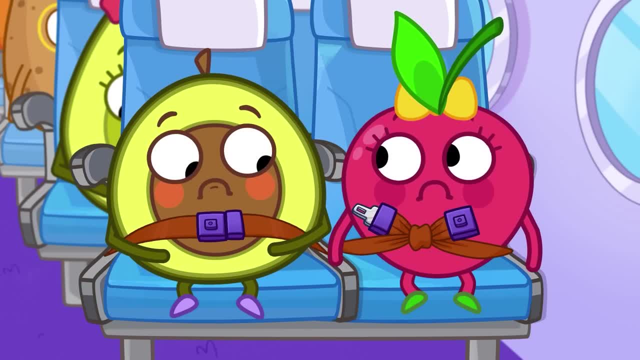 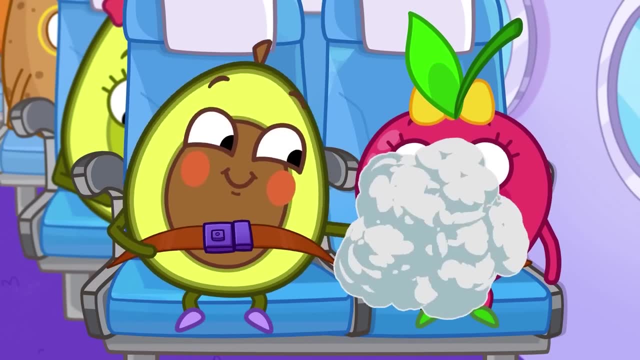 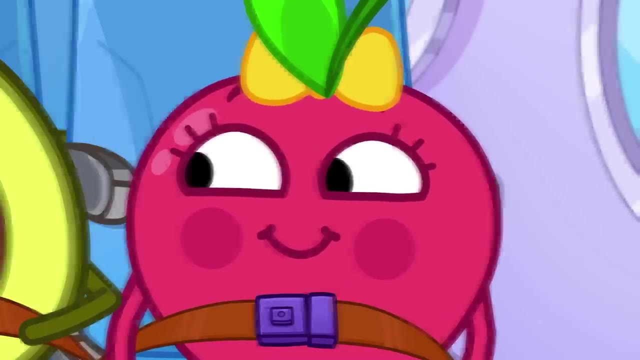 I So tired. I I yl. I might like to Rsr And you wanna get out of this house. Well, I'm afraid I'll leave without Lizzy. I don't know how we'll survive without her as well. 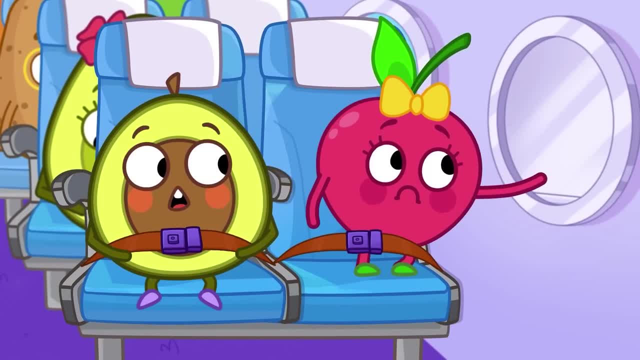 Who would let you leave fase menu, phase menu There, that's better, Koihick, Hoogaa-hoo, Whoa, wohoo, Whoa, whoo, Unh. Ah, that's so awkward, Hoogaaaaaa. 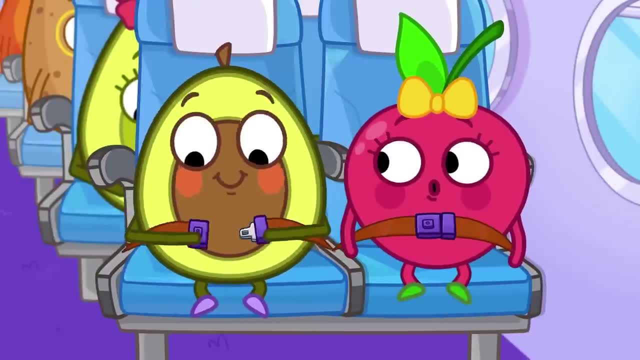 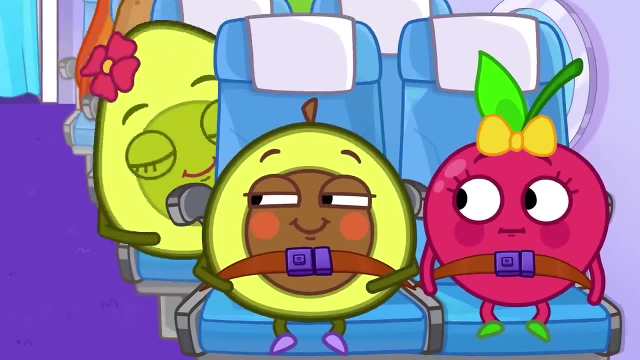 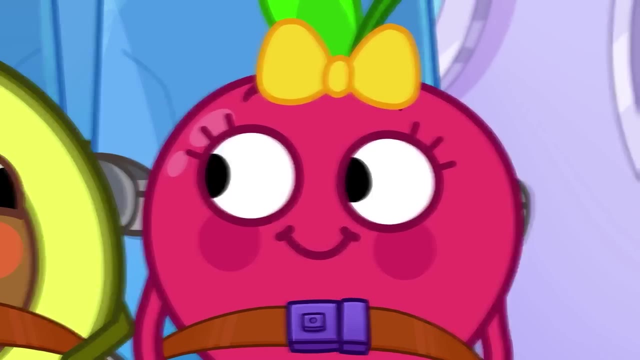 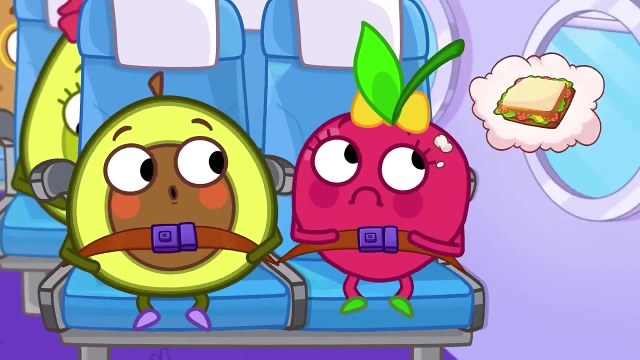 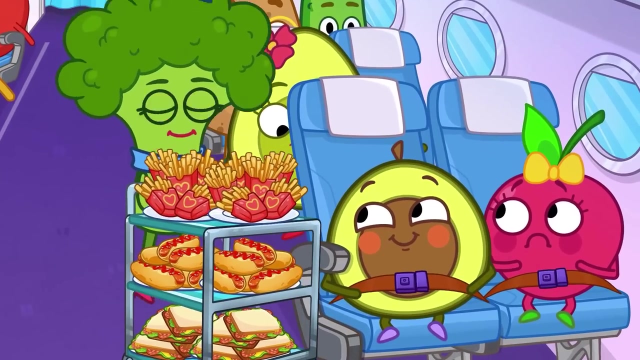 it. window blinds need to be open during takeoff and landing. am i right, mommy? you are right, honey. uh oh, cherry is very hungry. don't worry, everything you need is here, am i right? yes, you are pitt. the flight attendant has lots of food to choose from. 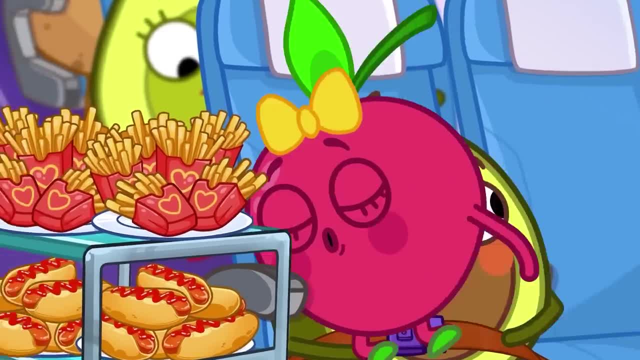 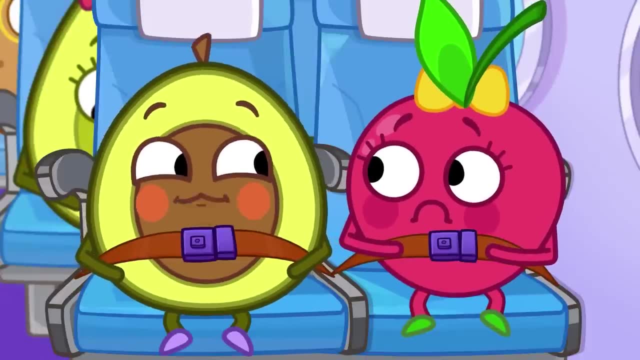 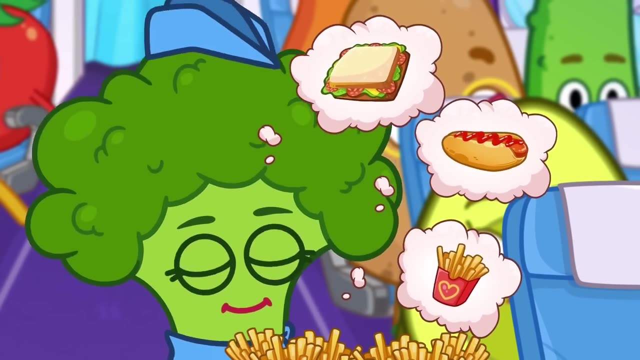 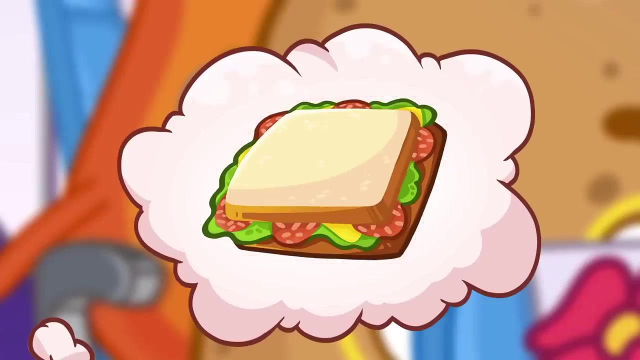 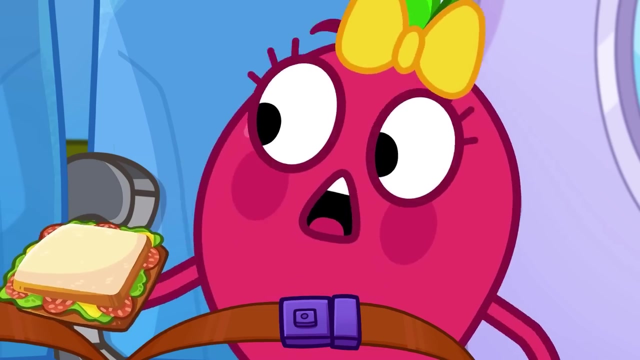 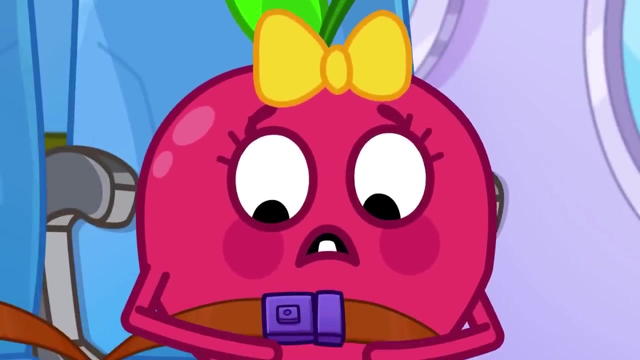 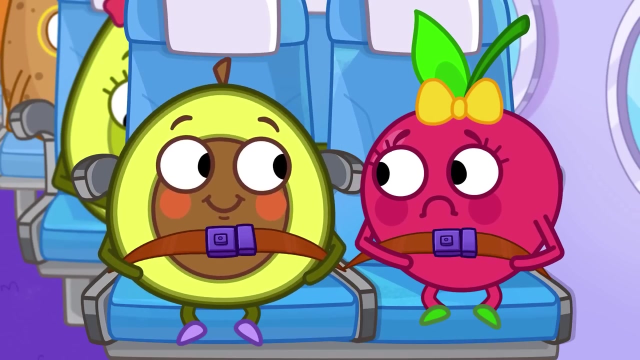 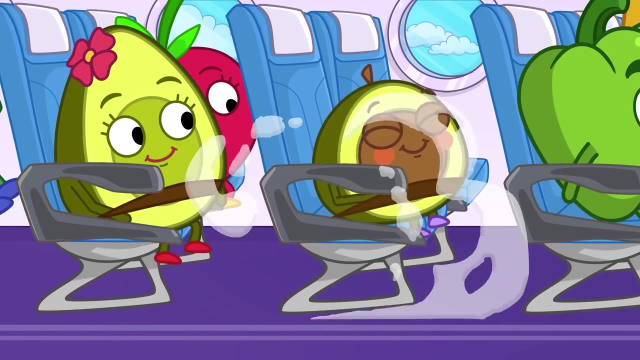 cherry, you must stay in your seat. if you need something, just ask. hmm, let's see what they have. what would you like to eat? she would like a sandwich, please. now, what's wrong? cherry needs the restroom. there's one at the back of the plane. the door is locked. 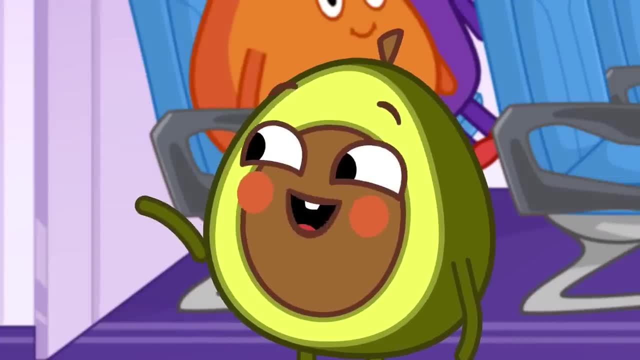 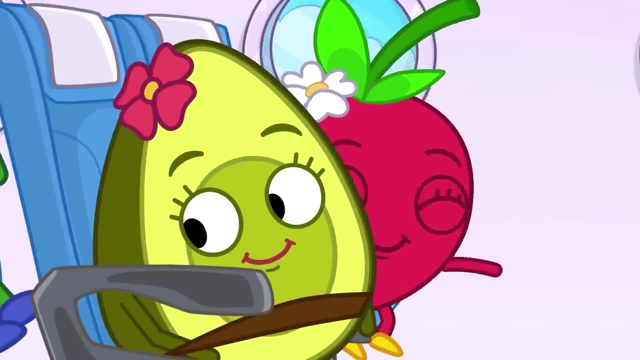 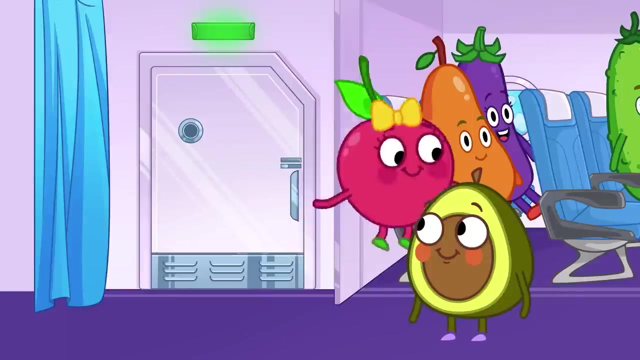 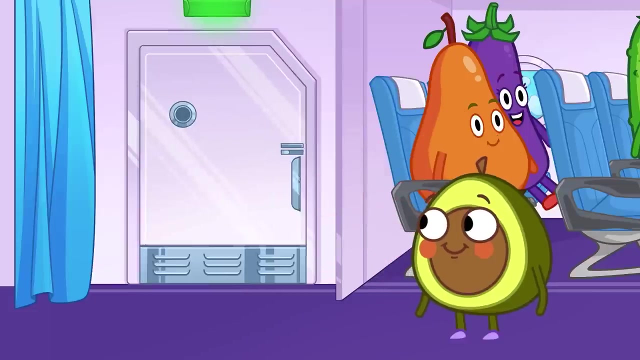 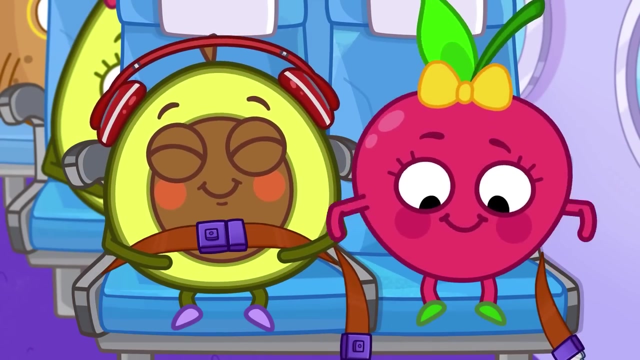 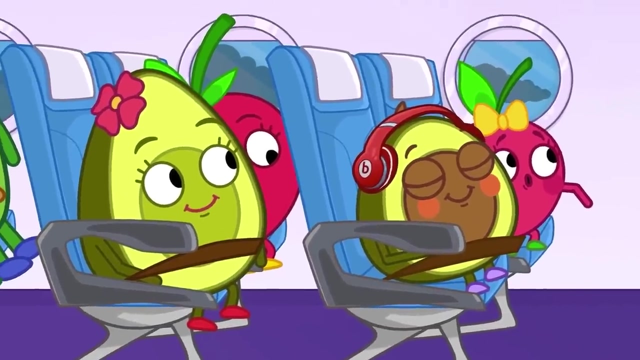 what does the red light mean? pitt, if this sign is red, the toilet is occupied. am i right? of course you just have to wait your turn now. cherry can use the restroom. hold on the flight is about to get bumpy, cherry. what's wrong? i'm scared. don't be afraid, honey. 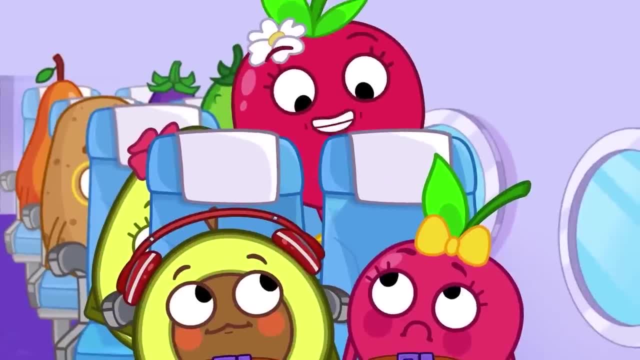 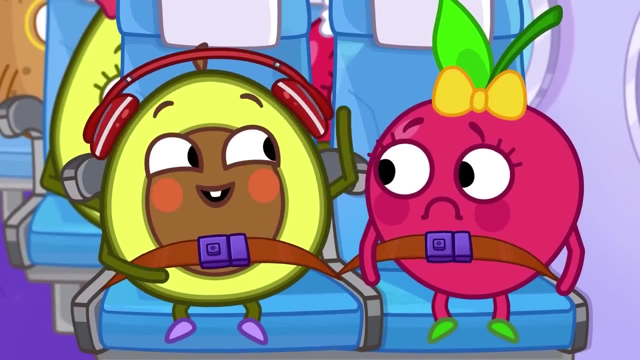 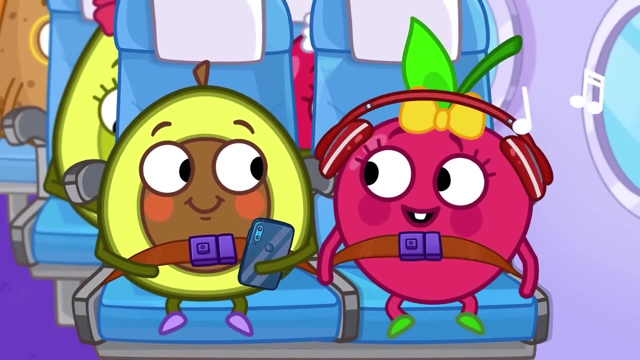 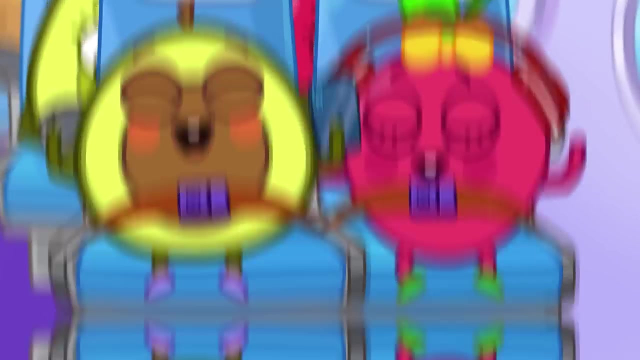 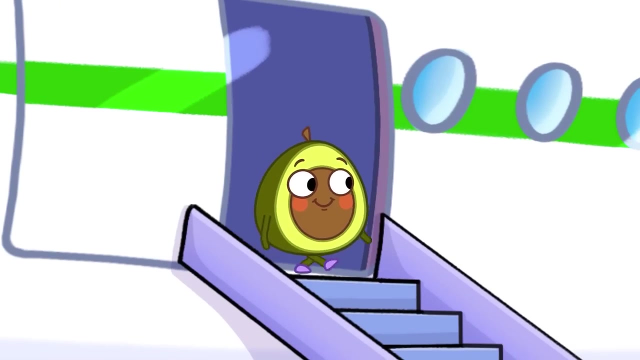 cherry, what's wrong? i'm scared. don't be afraid, honey, it's just tubulence. don't be afraid, honey, it's just tubulence. don't be afraid, honey, it's just tubulence. music will make you feel better. music will make you feel better. see, cherry, there was nothing to worry about. 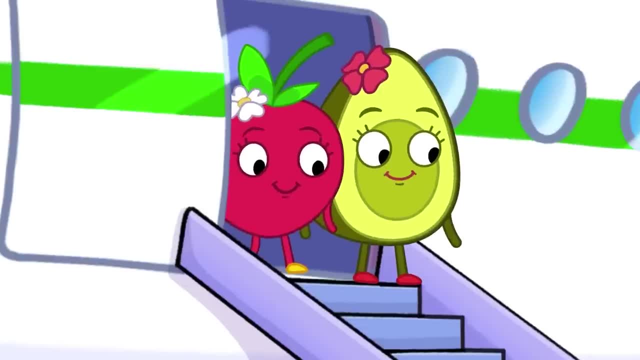 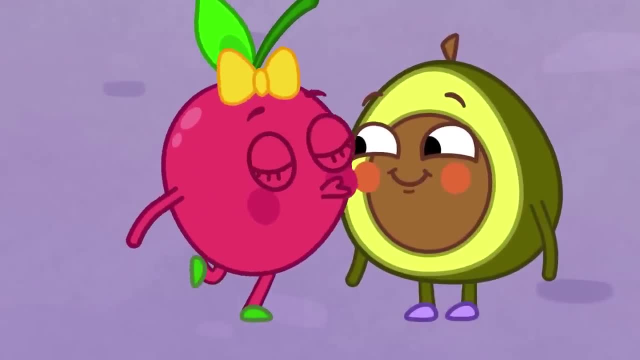 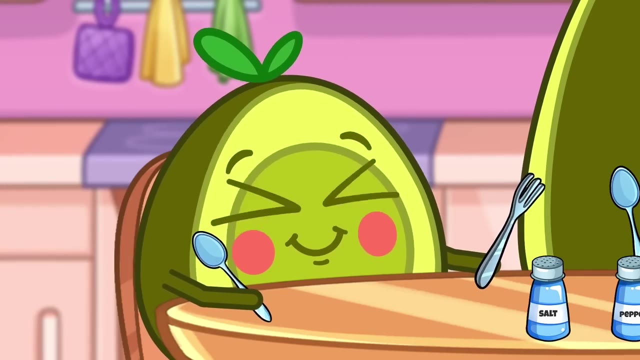 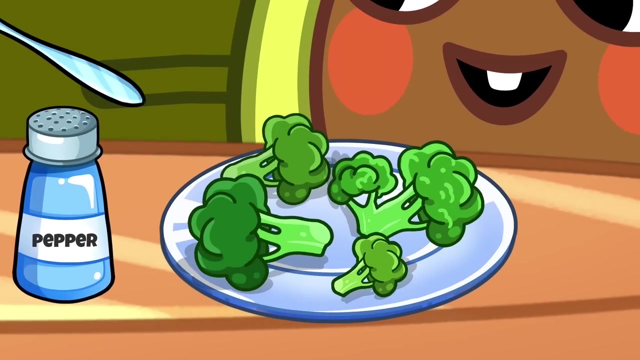 music will make you feel better. i won't be afraid of flying anymore, thank you. music will make you feel better. have fun, kids. music will make you feel better. hello penny, hello pitt. what has mommy made for lunch? it's broccoli yum. music will make you feel better. 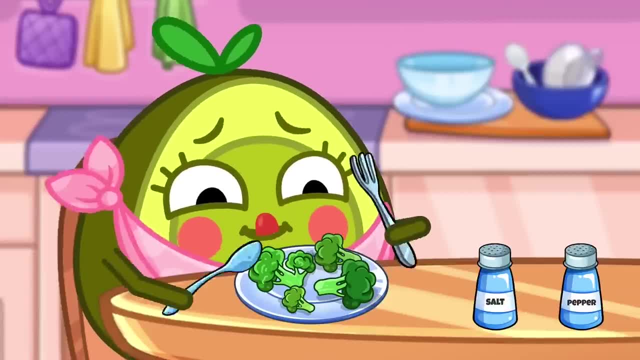 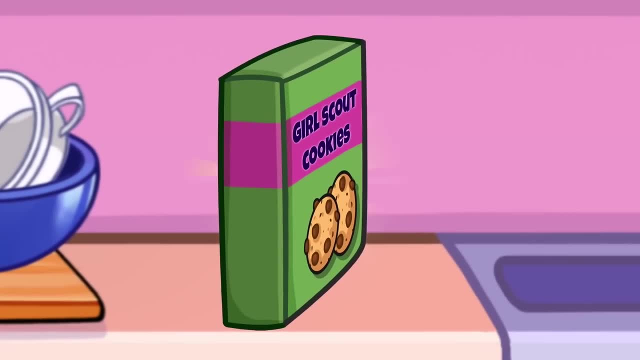 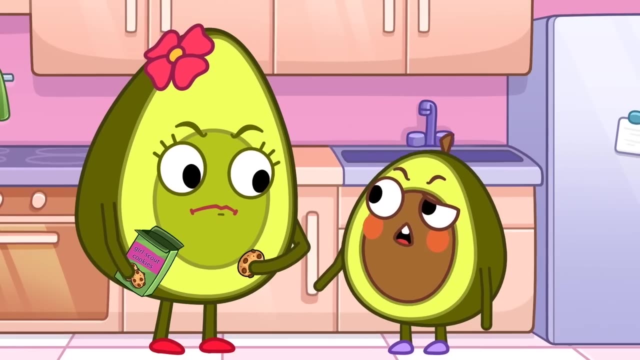 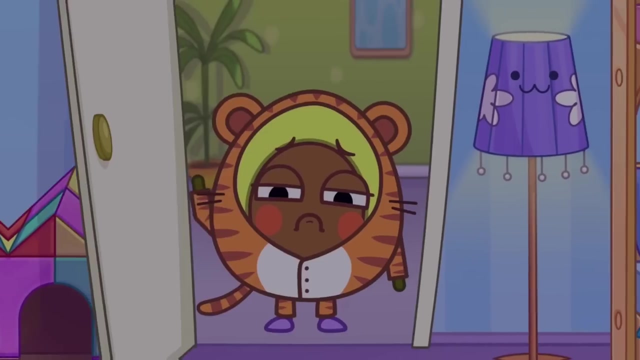 music will make you feel better. penny loves vegetables. penny loves vegetables. pitt does not. he'd rather eat cookies. wait, pitt, did you ask mommy first? pitt, you should eat vegetables to stay pitt. you should eat vegetables to stay pitt. you should eat vegetables to stay healthy. 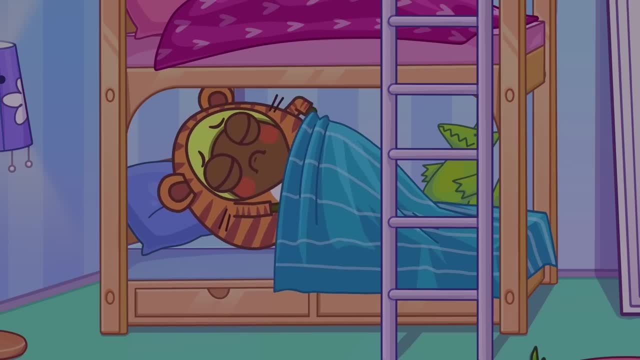 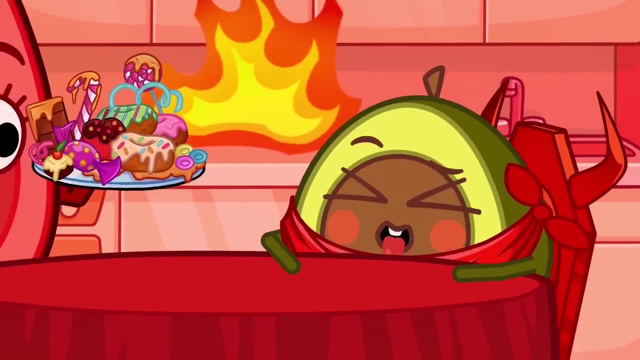 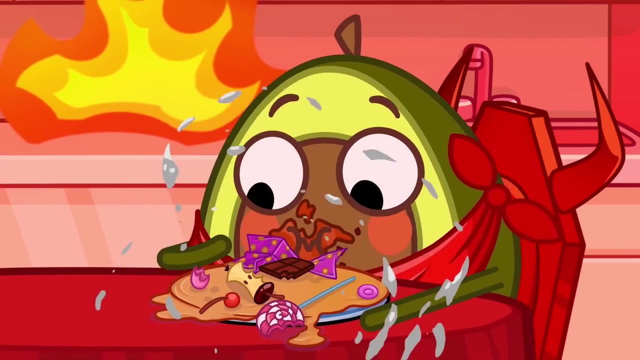 do, do, do, do, do, do, do. let's see what pitt is dreaming about. let's see what pitt is dreaming about. let's see what pitt is dreaming about. dream mommy is serving sweets for lunch. dream mommy is serving sweets for lunch. dream mommy is serving sweets for lunch. so much junk food will give you a tummy. 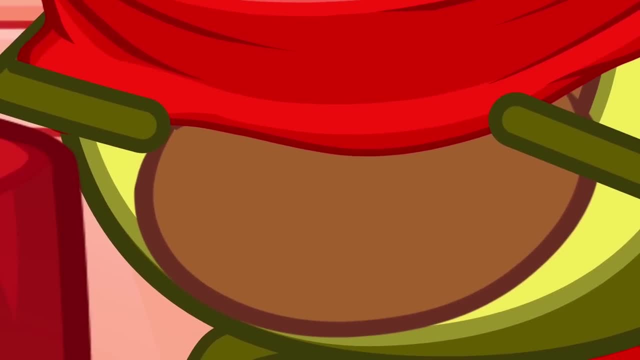 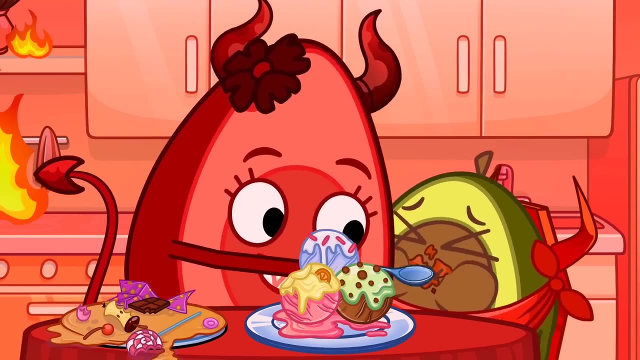 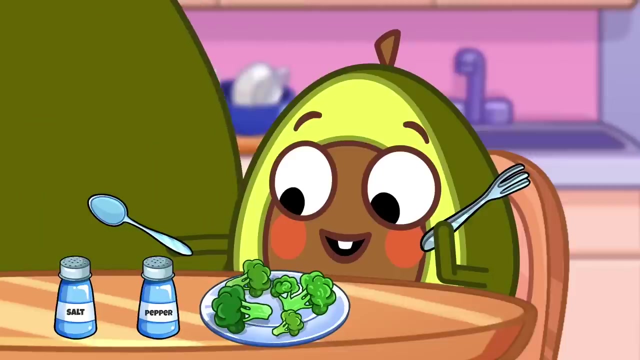 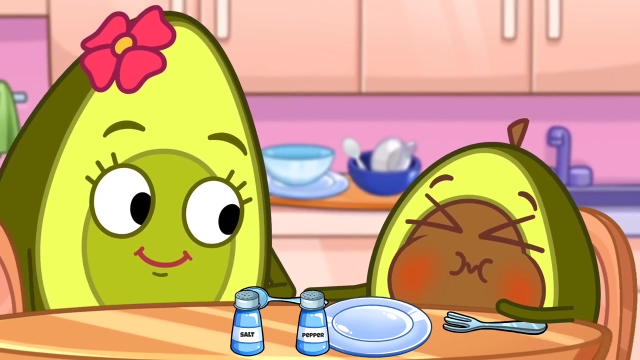 so much junk food will give you a tummy. so much junk food will give you a tummy egg. mommy, my tummy hurts. mommy, my tummy hurts. mommy, my tummy hurts. Will Pit eat his broccoli today? Good job, Mommy, is so proud of you two. 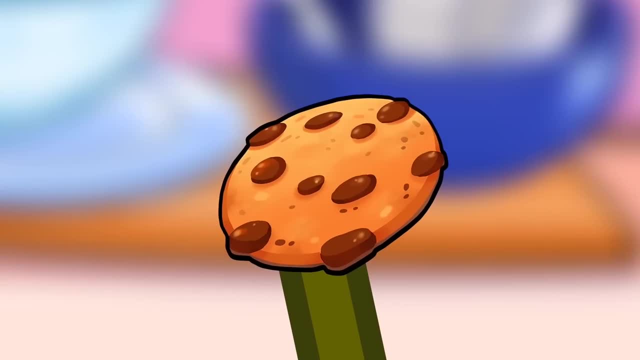 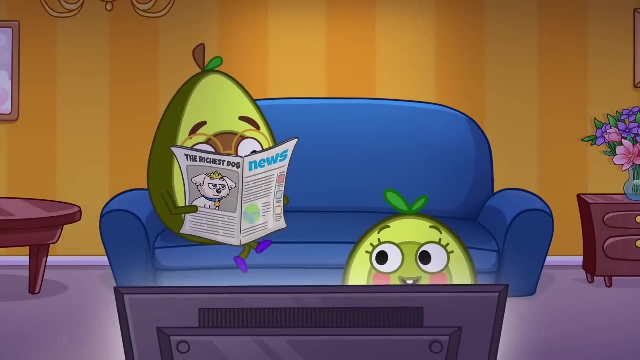 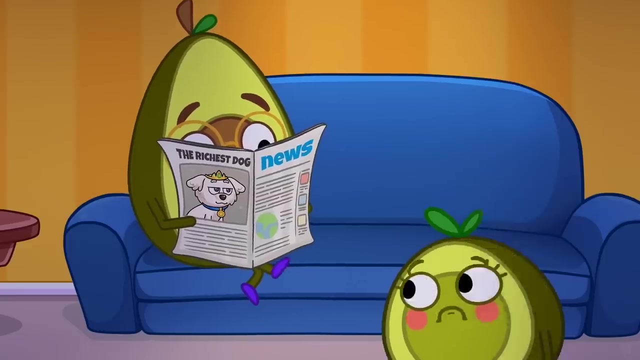 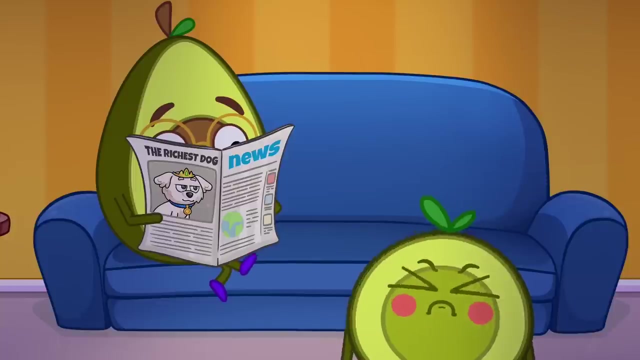 Well done, Here's your cookie. Thank you, Mommy. Penny is watching her favorite show. Penny, you're sitting too close to the TV. Hmm, hmm, hmm, hmm, beeeep. Hmm, hmm, hmm, hmm, haaaah. 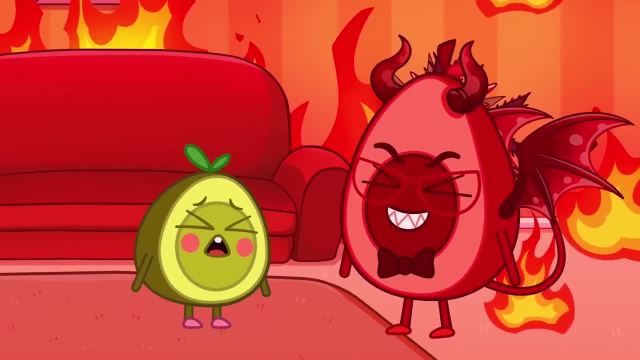 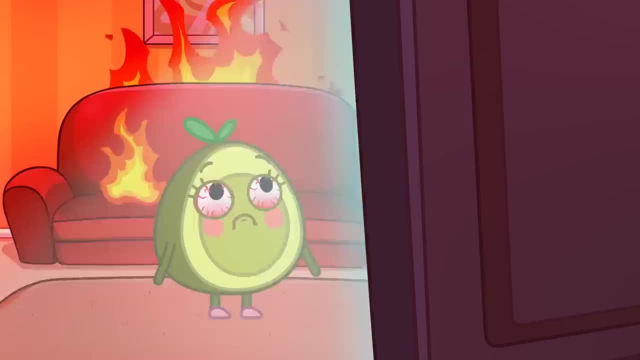 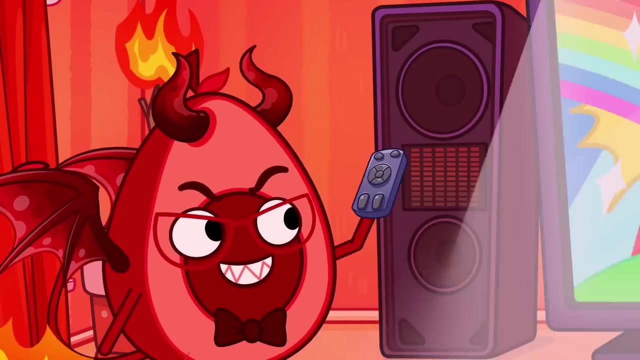 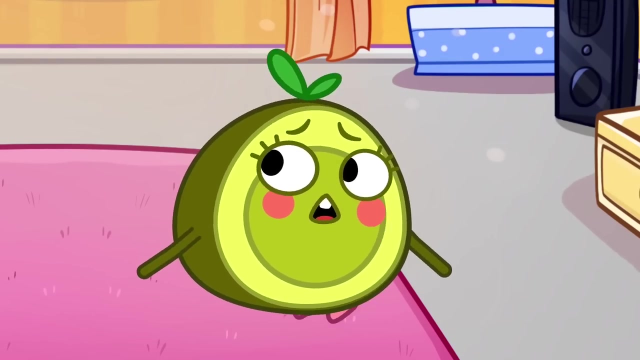 Let's see what she's dreaming about. Uh-oh, What is Dream Daddy? up to Careful, Penny. Being too close to the TV is not healthy, Daddy. my eyes hurt. Hehehehe, Penny, maybe you should sit beside Daddy. 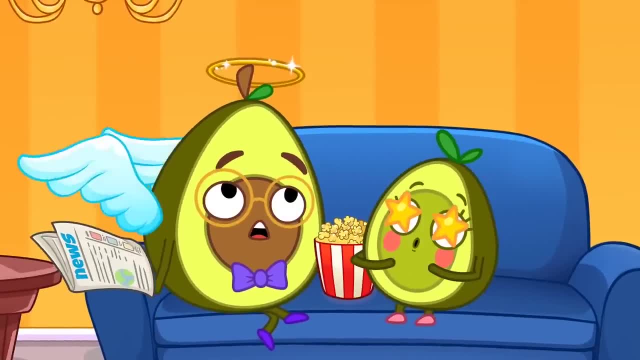 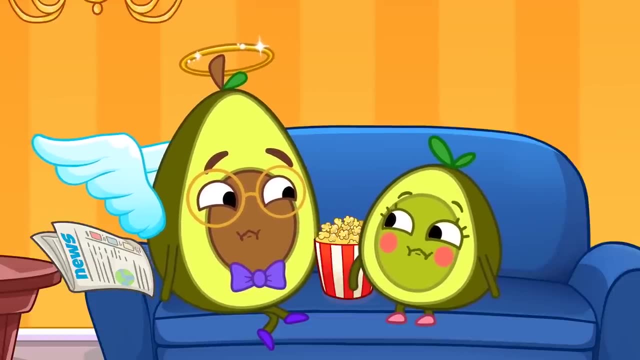 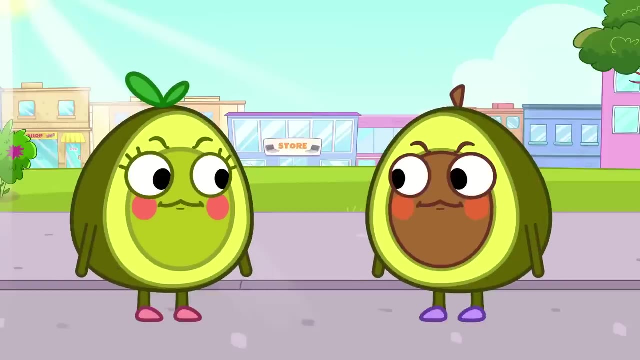 He might even share his popcorn. Let's watch a movie together. Thank you, Daddy. Pit and Penny have found a maze And there's a special prize inside. Hehehehe, Who will find the prize first? Oh, Green, red, blue. 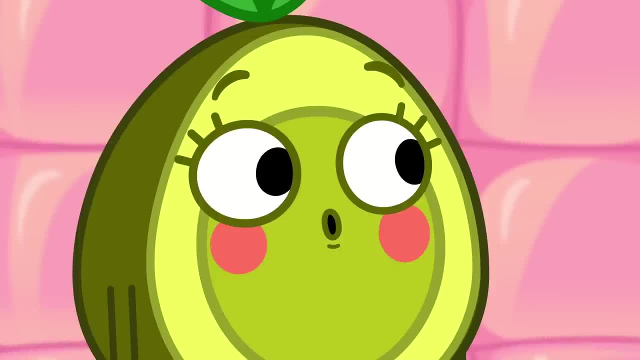 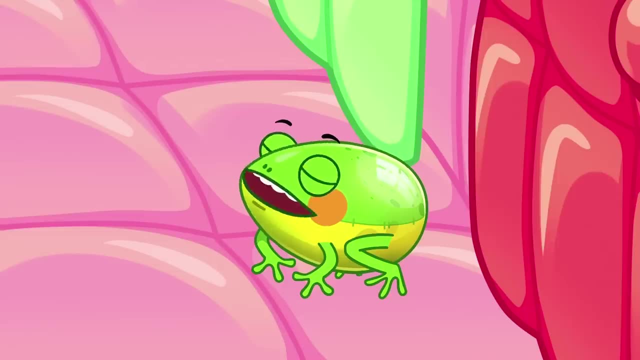 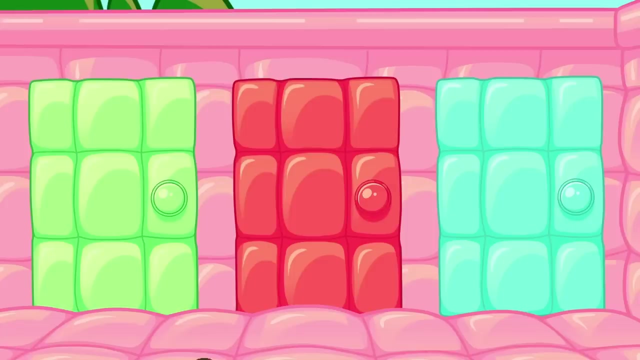 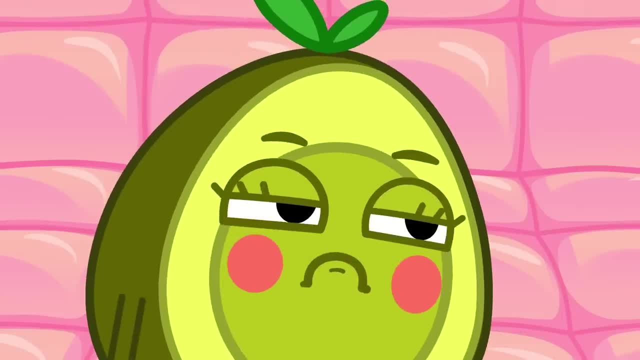 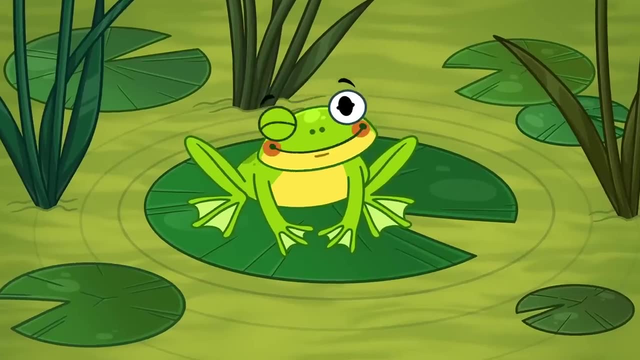 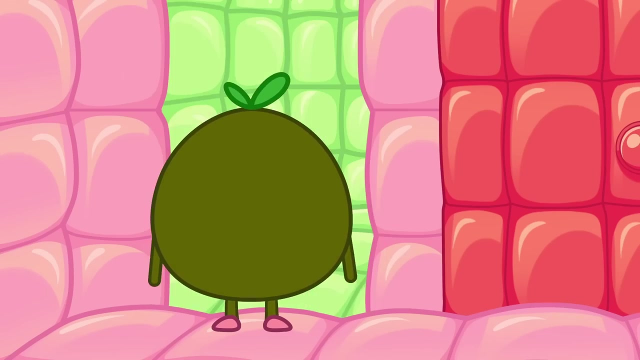 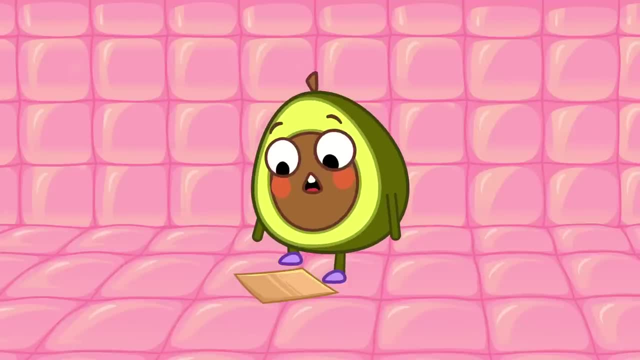 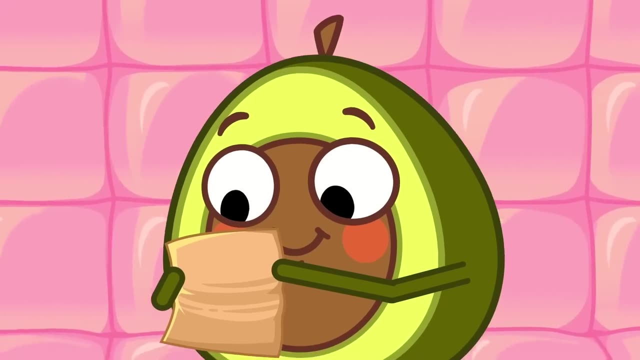 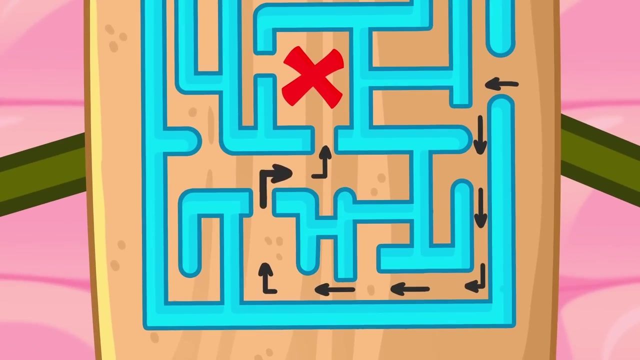 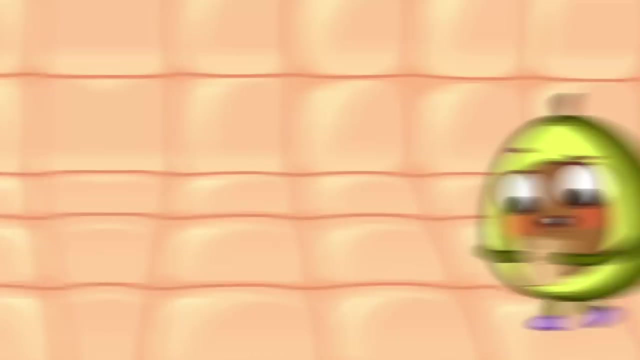 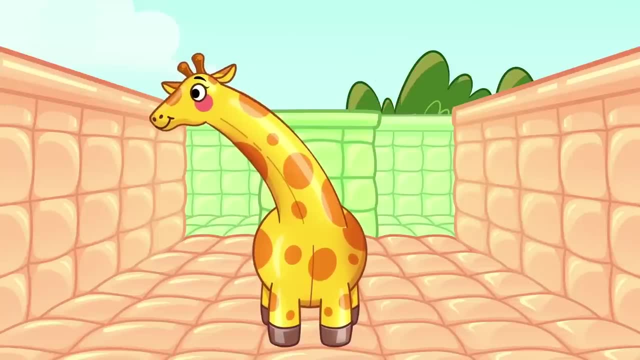 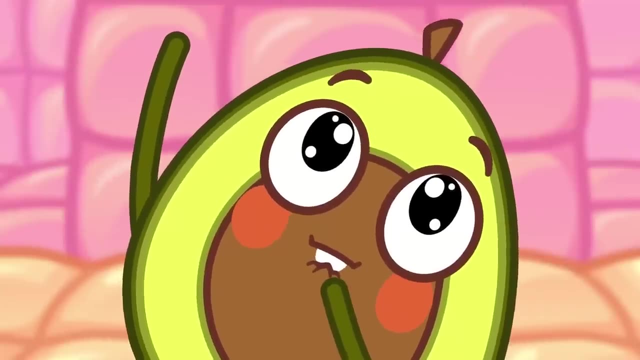 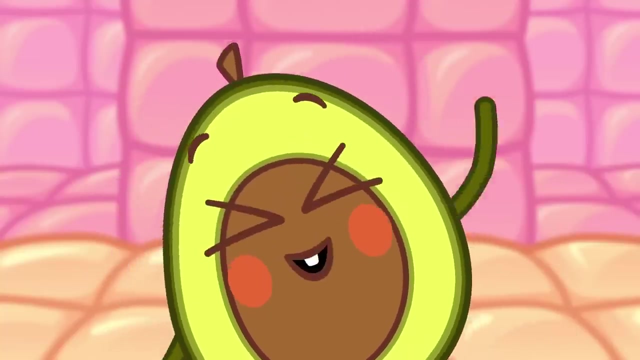 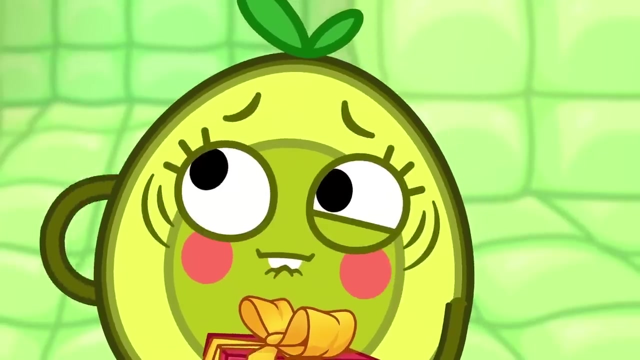 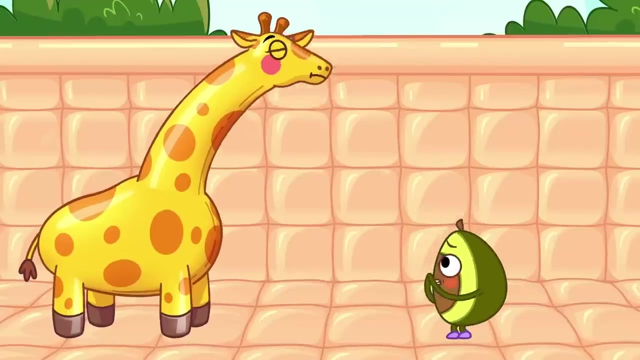 Right Left, Right, Left, Left. Hmm, what does Mr Draft think? Right Left, Penny found the prize, But which door is the exit? Pit Pit, Mr Draft, can you see Penny? She's right over there. 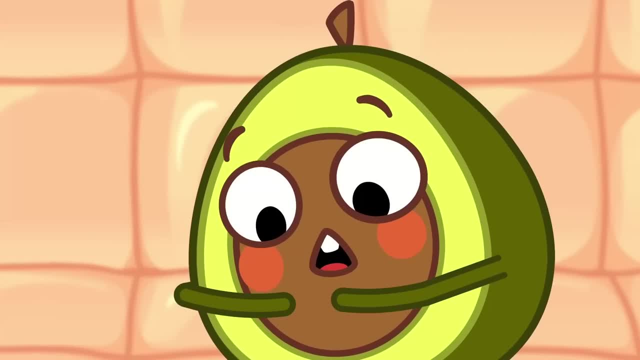 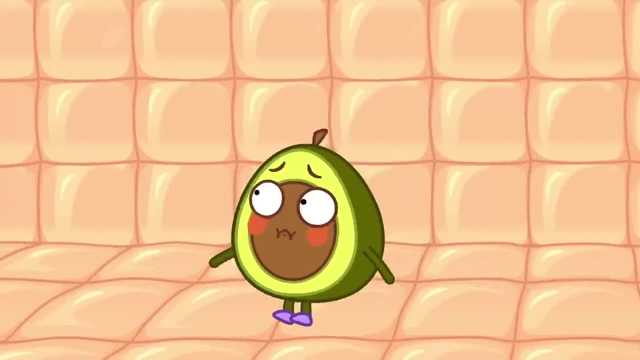 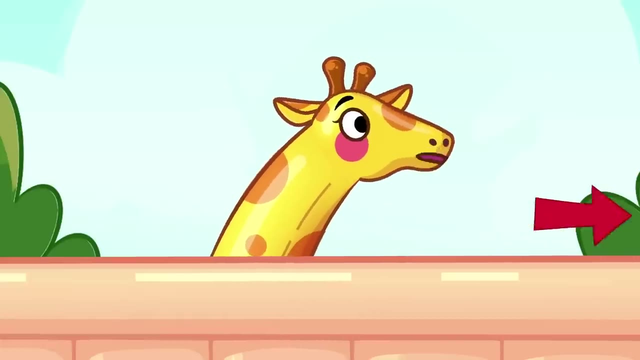 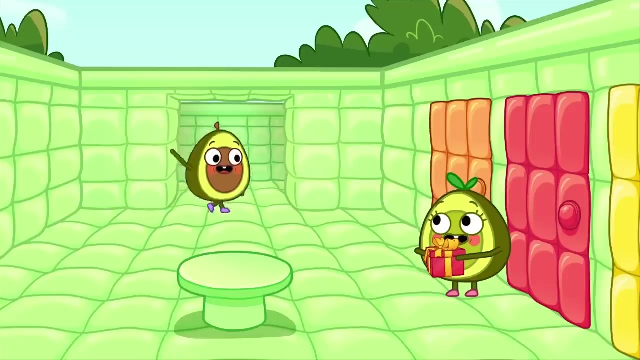 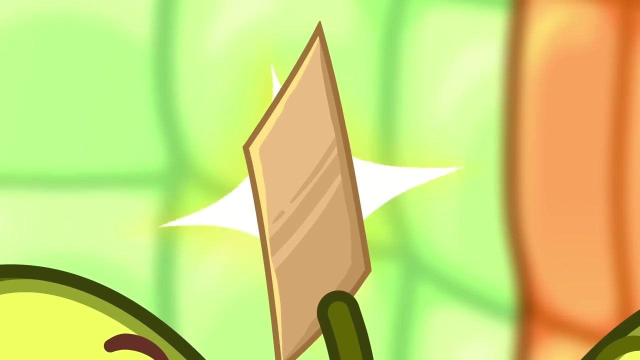 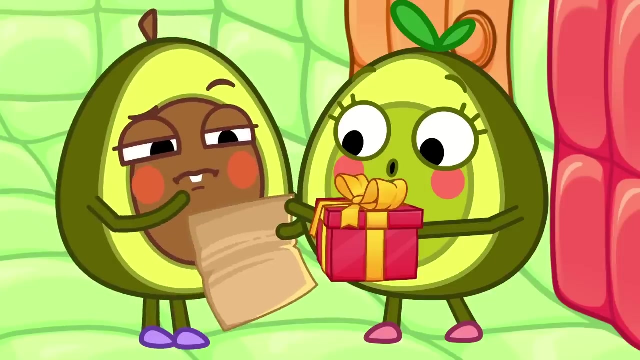 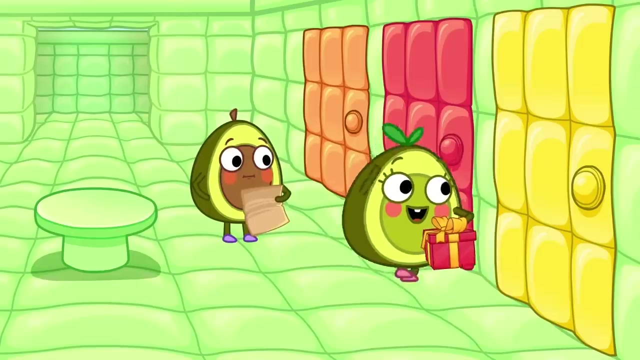 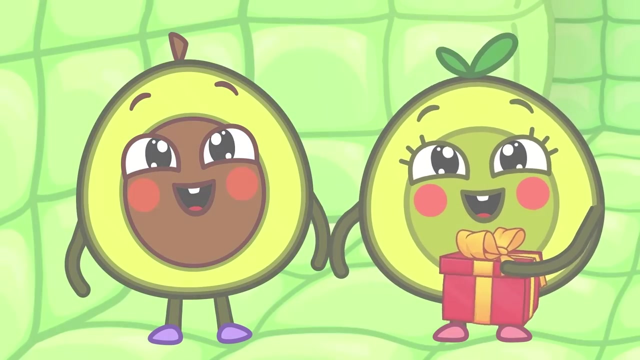 Left Pit. which way is left Correct? Now, which way Right? You can do it. Pit, Pit, Pit. Maybe the map shows where the exit is. Do you see it? Yes, Which door is the exit? Pit and Penny made it through the maze. 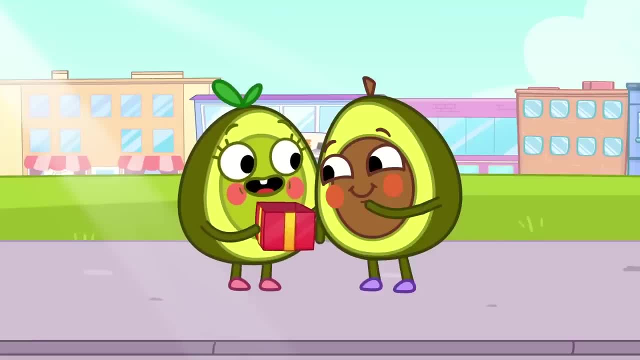 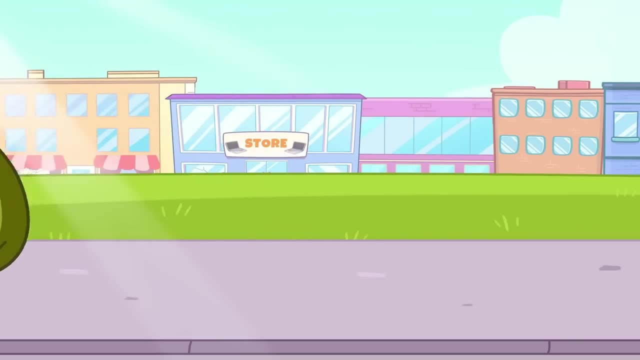 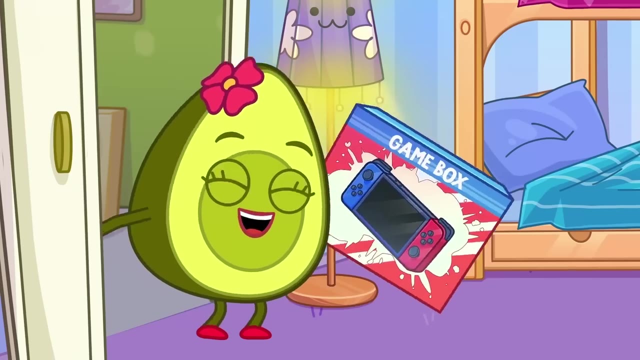 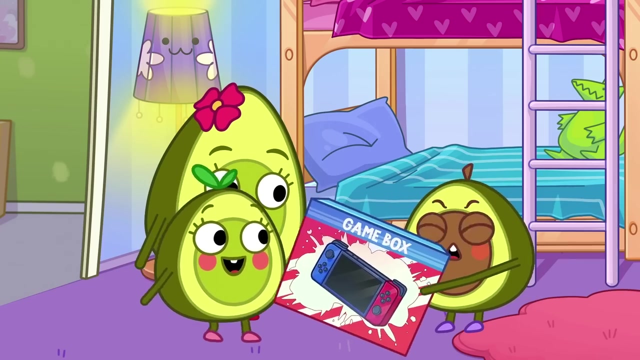 Yes, Yes, Yes. But what is the prize? Two pop-it toys. Have fun, kids, Pit and Penny. Mommy has a surprise for you. It's the new game box Fun, But Pit and Penny don't want to share. 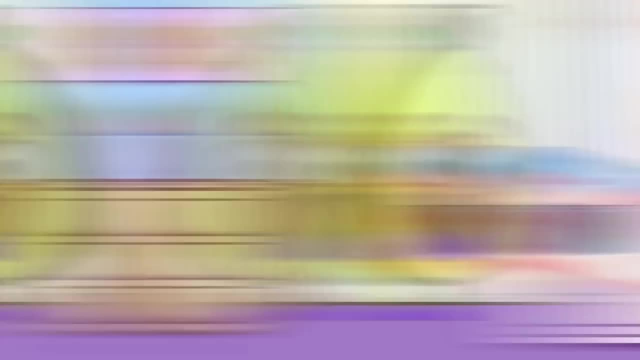 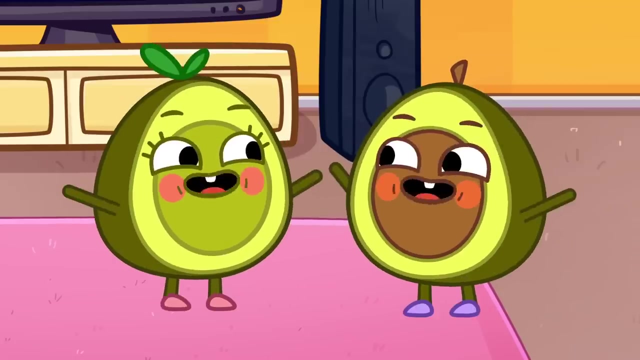 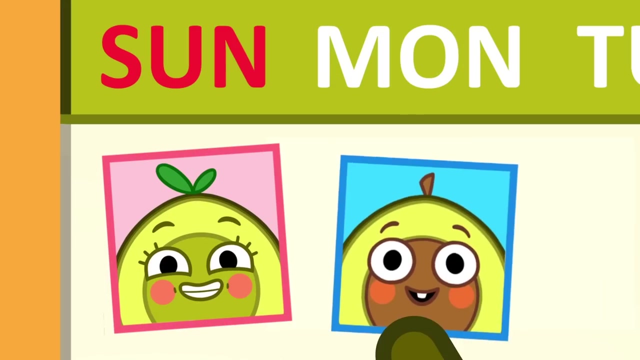 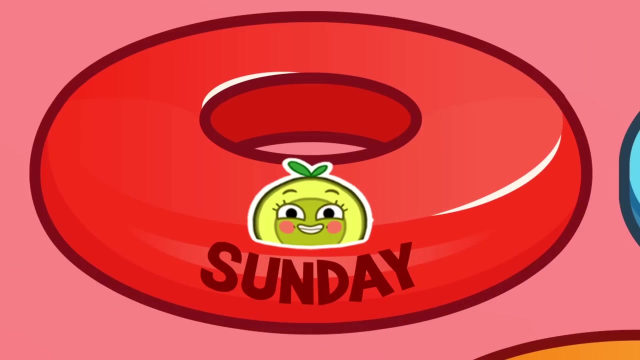 Oh, no, Good catch. Daddy Pit and Penny need to take turns. What day is this Sunday? On Sunday, Penny gets the game box Monday And Pit gets it on Monday. Hmm, Aha, What day is it, Penny? 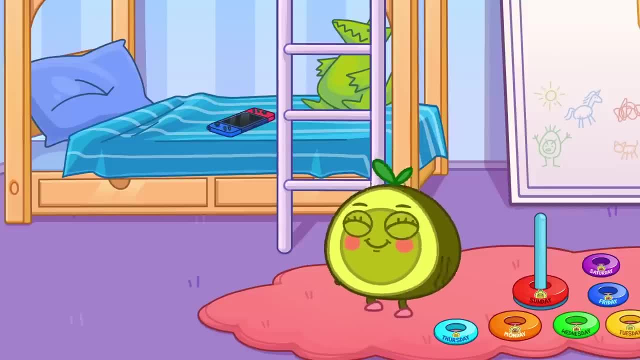 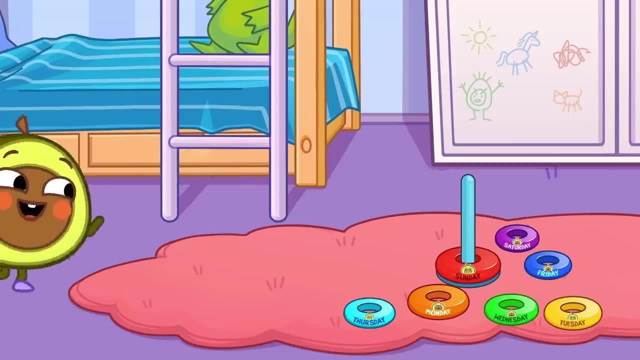 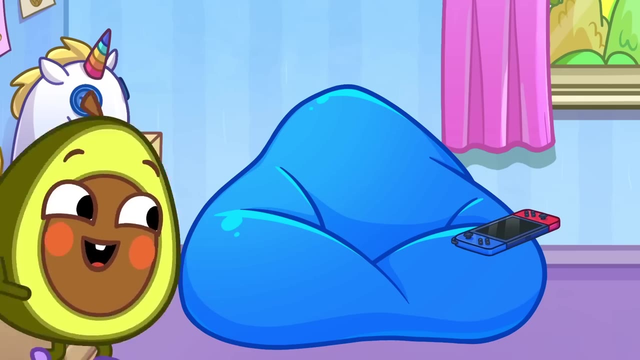 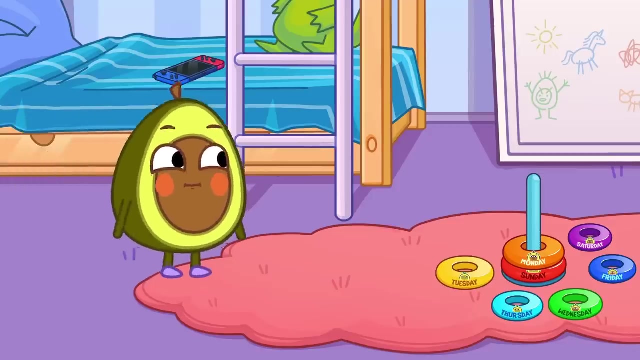 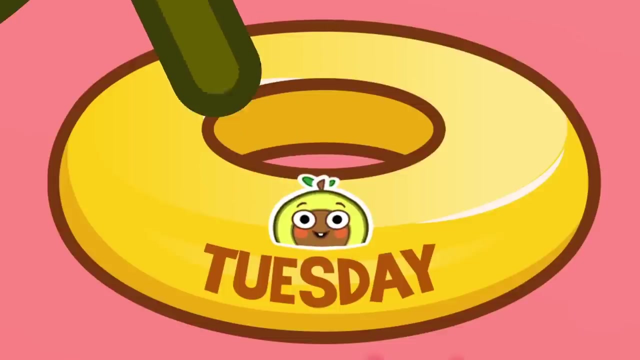 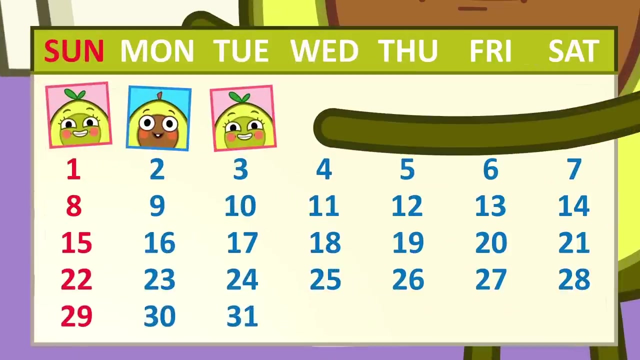 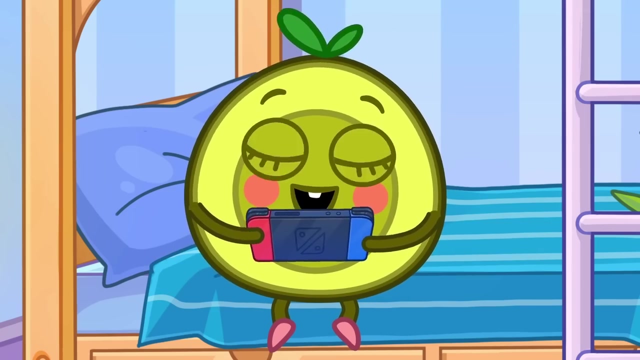 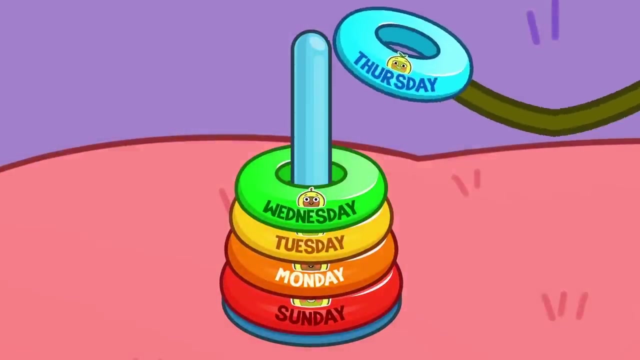 Sunday: What day is it? Pit Monday? What are you up to Pit Tuesday? But Pit, it's not your turn. Ahem, It's Penny's turn on Tuesdays. Okay, Yay, Wednesday, Thursday. 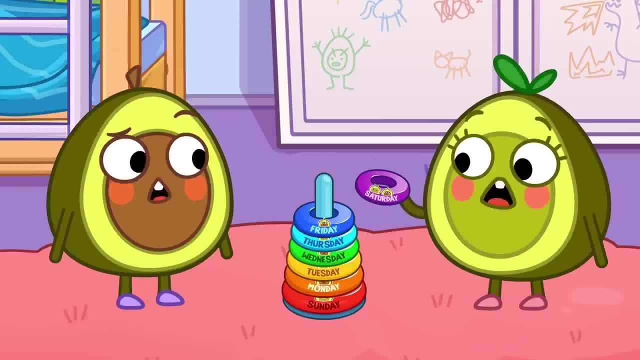 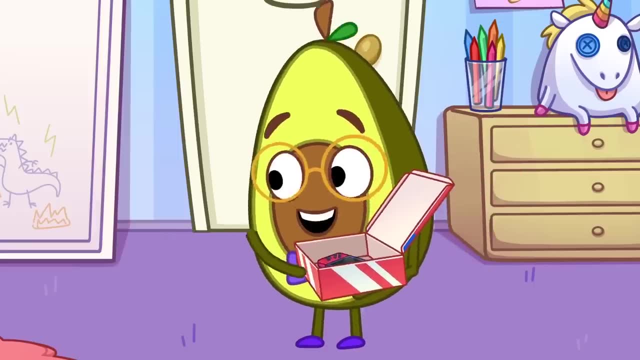 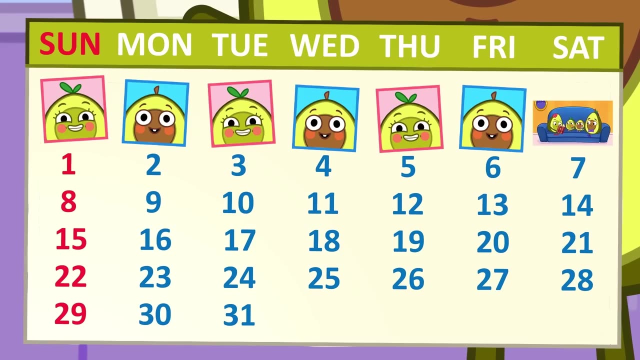 Friday, Saturday. Now what are Pit and Penny to do? Ahem, Why did Daddy put the game in a box? You've learned all the days of the week Good job. Saturday is a family day, Blah-blah-blah-blah. 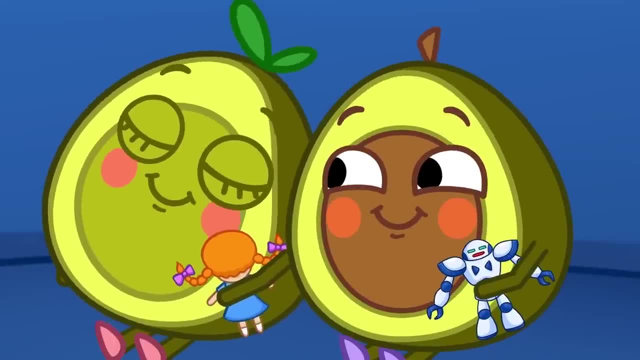 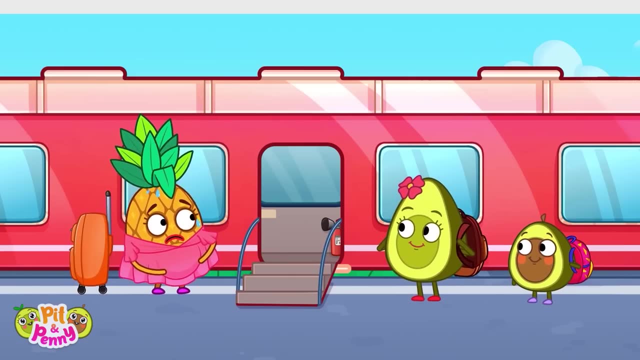 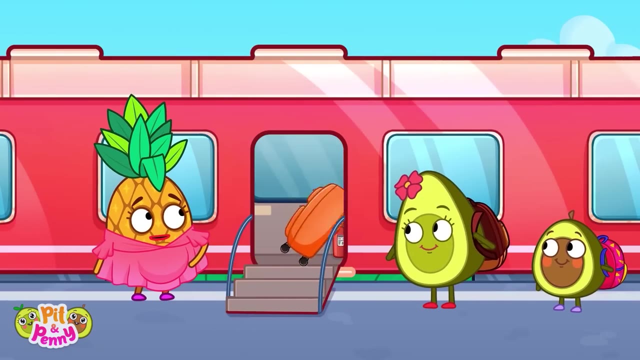 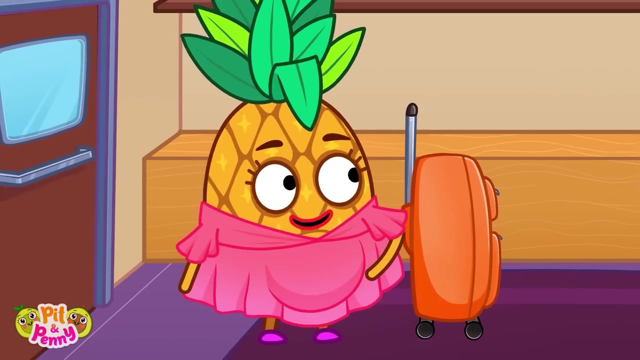 Blah-blah-blah-blah. It's nice to spend time with family. Have fun. Pit and Mommy are taking the train. Can someone help Miss Pineapple with her luggage? Thank you, Miss Pineapple needs more help with her luggage. 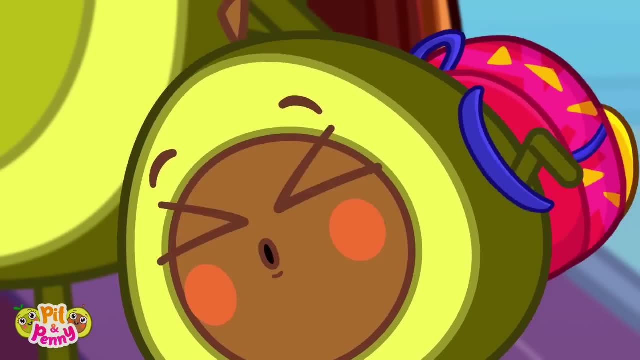 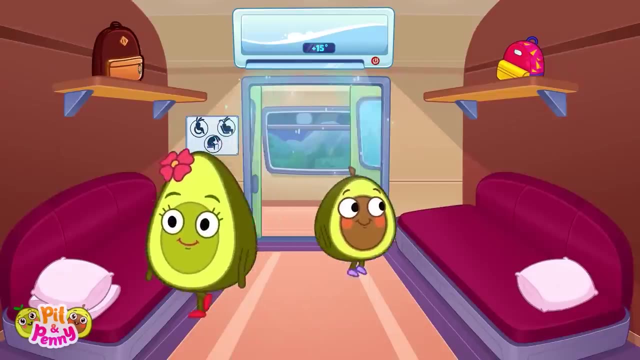 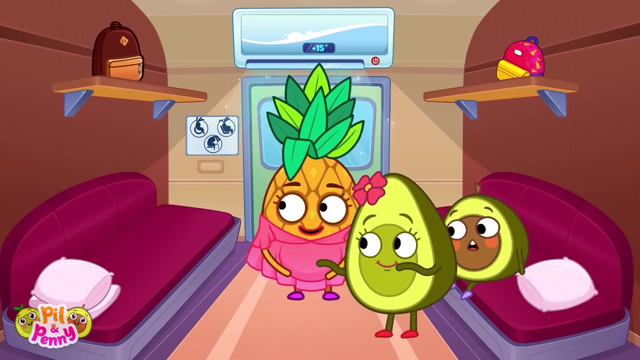 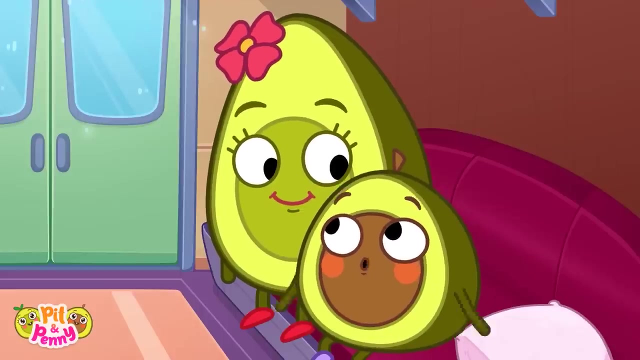 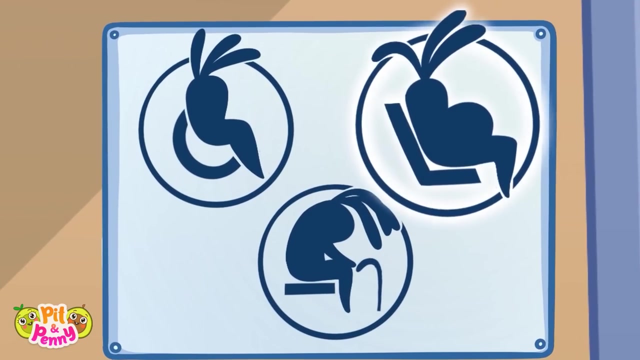 Oh, thank you. Hurry time to find your seats. Look at all the room you have. Mommy gives Miss Pineapple her seat. Thank you, Mommy. Why does everyone help this woman? This sign shows the kinds of people who might need extra help. 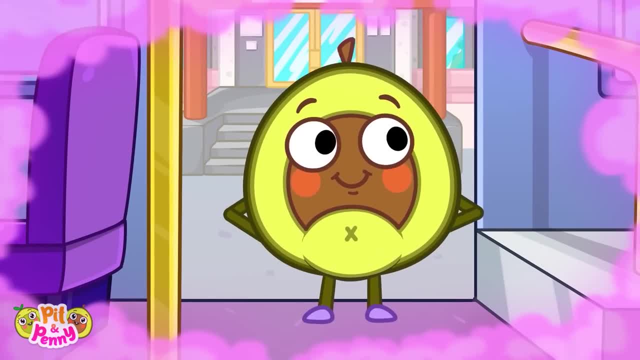 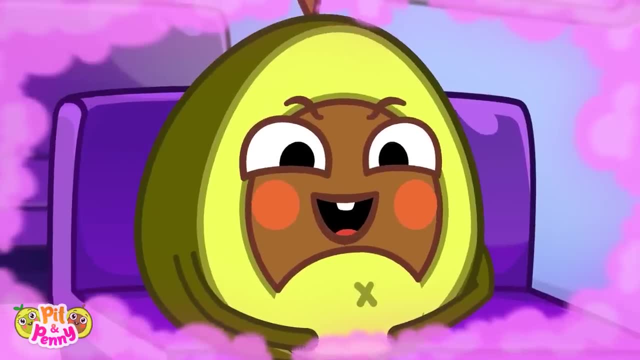 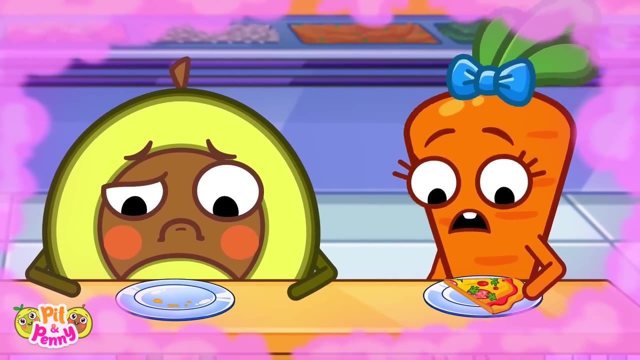 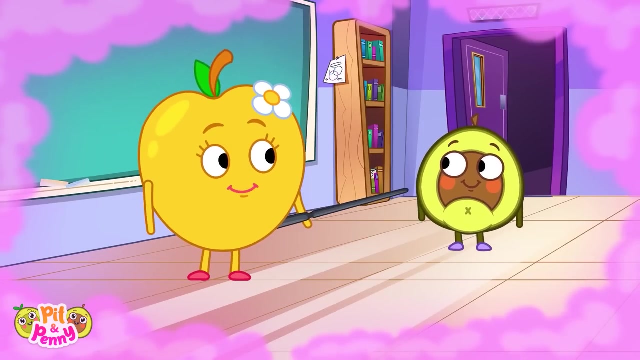 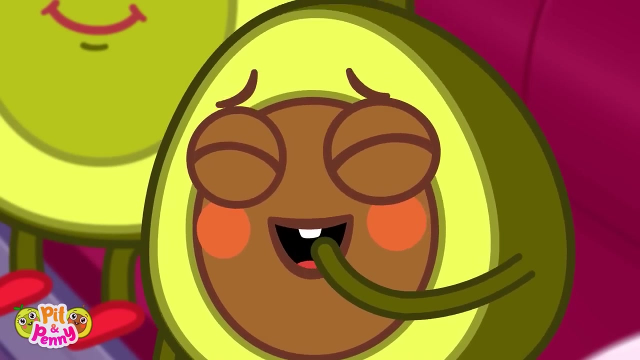 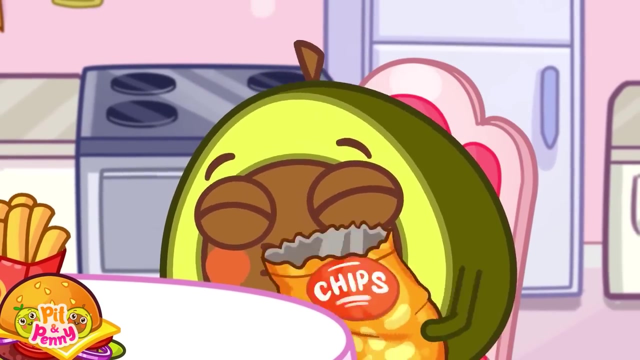 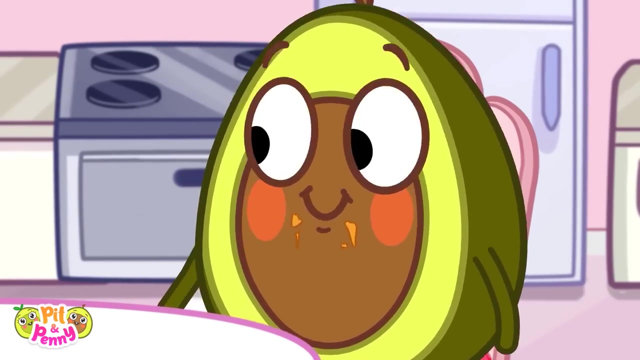 Hidden, Who imagines what would happen if he had a big belly. Now people will give him their seat And give him their food And give him their job Pit. that's not a very healthy lunch. All that junk food is bad for you. 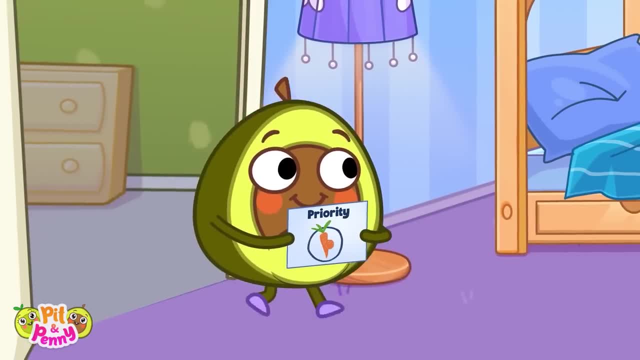 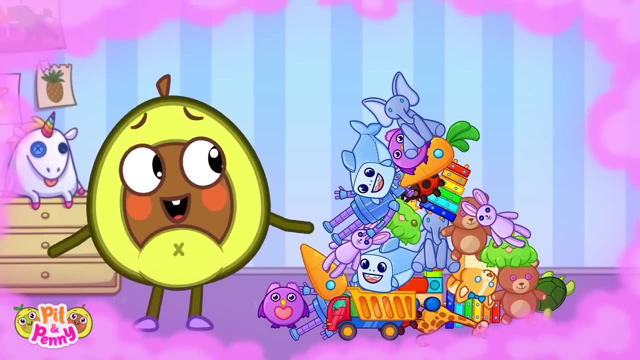 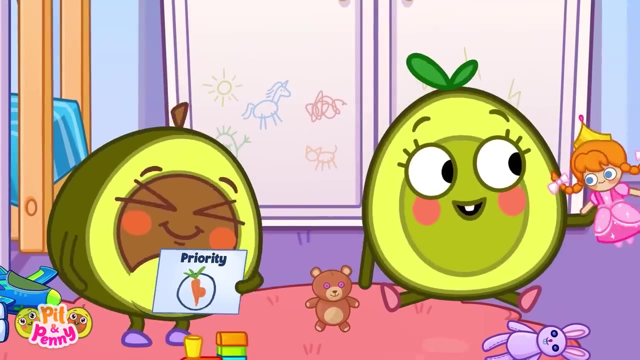 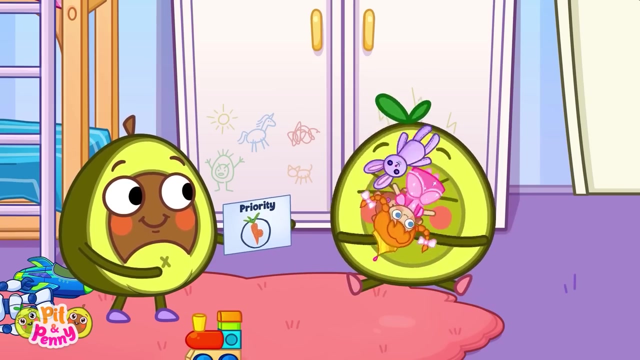 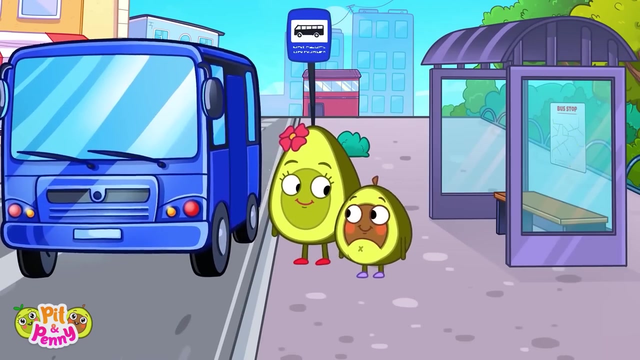 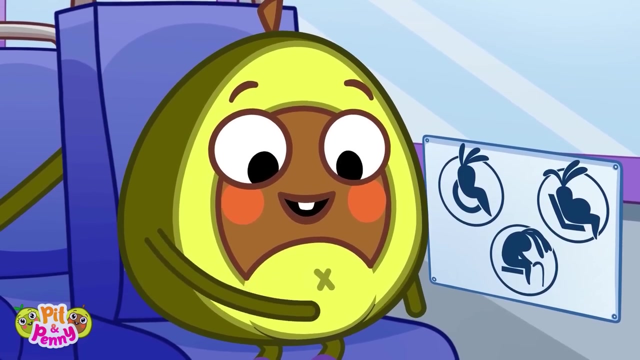 Pit. look at your belly. Oh Pit Pit. What does Pit want? now Give me your toys. Sorry, Pit, Pit, Pit and Mommy are talking. Pit and Mommy are taking a bus. Oh hello, Mrs Pineapple. 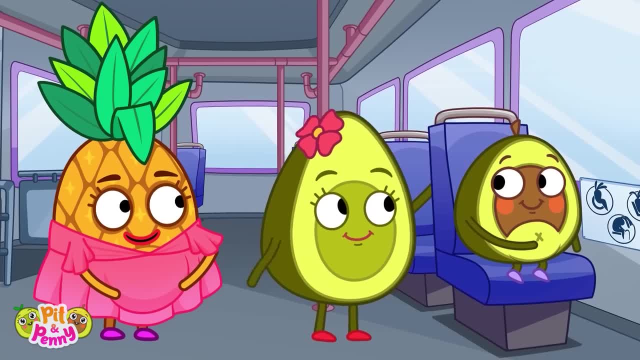 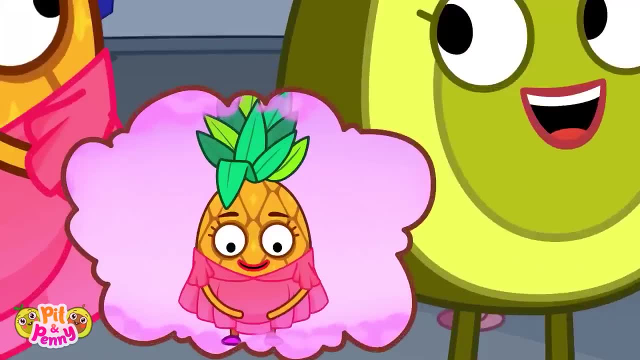 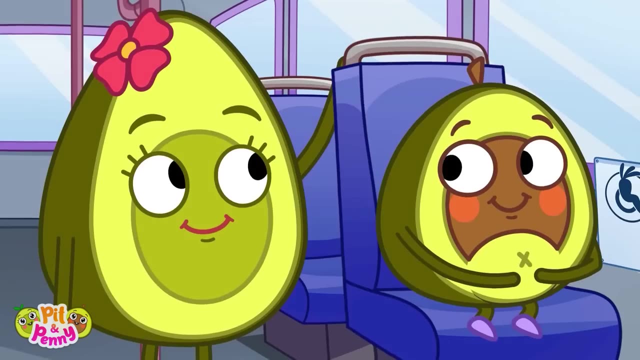 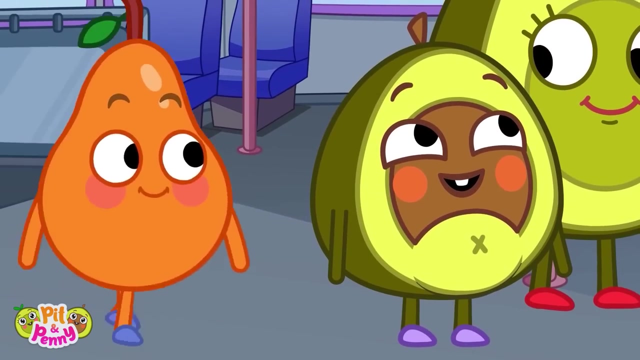 Pit give up your seat for Miss Pineapple, please. Why not, Pit Pit? Miss Pineapple has got a baby in her belly. She's pregnant. Pit gives Miss Pineapple his seat. Thank you, Pit. How kind. 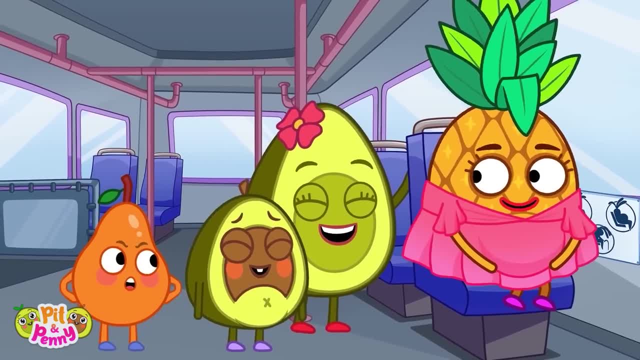 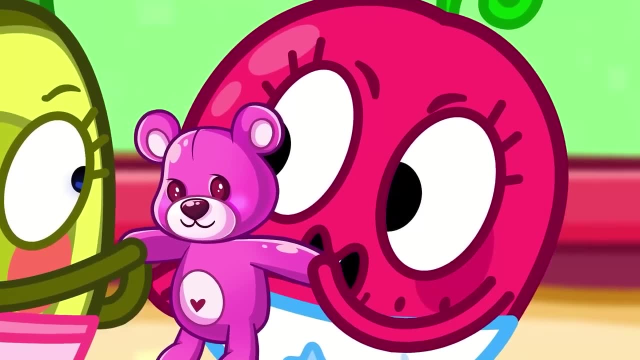 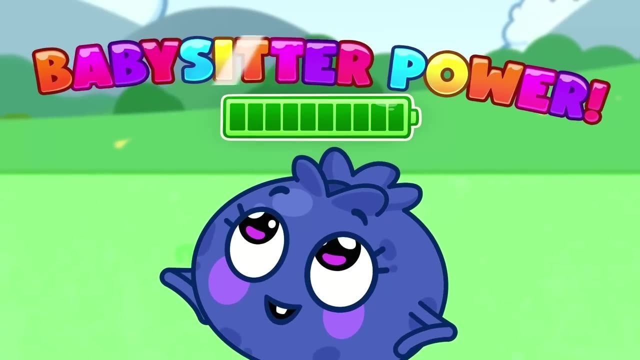 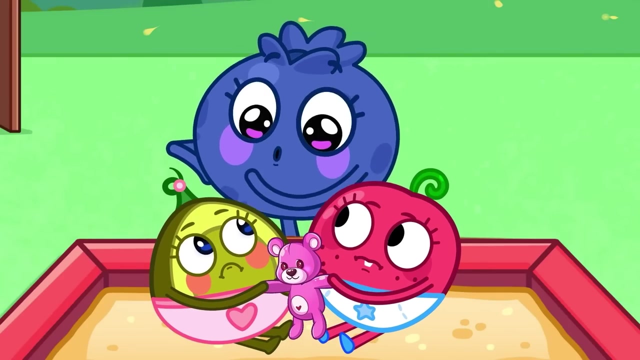 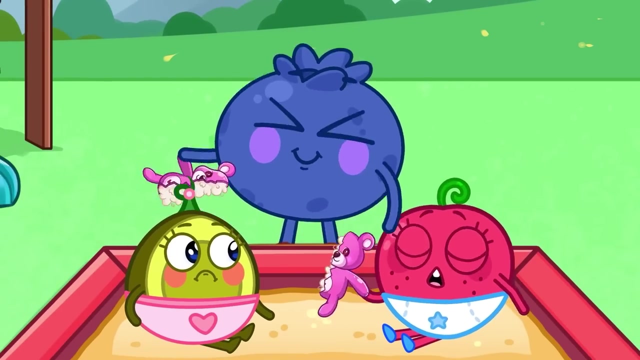 But Pit isn't pregnant, He just ate too much. Baby Avocado and Baby Cherry are fighting over the teddy bear. Maybe Blueberry can help. She'll use babysitter power. I'll help you. Blueberry didn't help Because Mr Pineapple doesn't like her pretty face. 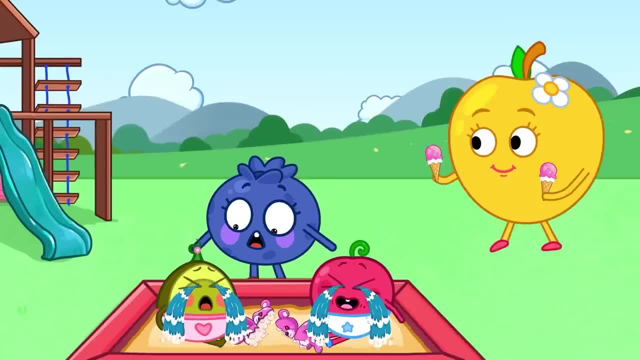 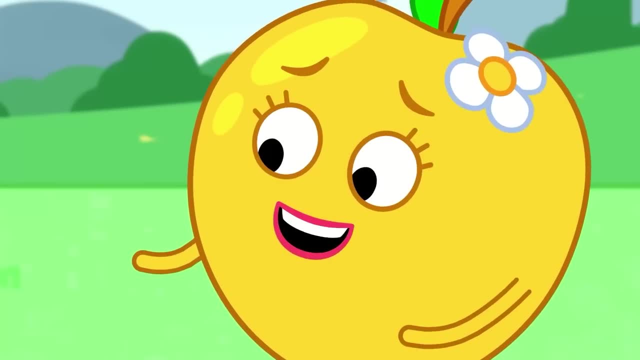 Oh Wow, I love you Blue. So happy for you, I'm so happy. Will you get me a coffee Pit? I will. I love you Pit. Oh, Blueberry, That didn't help. Who is it? 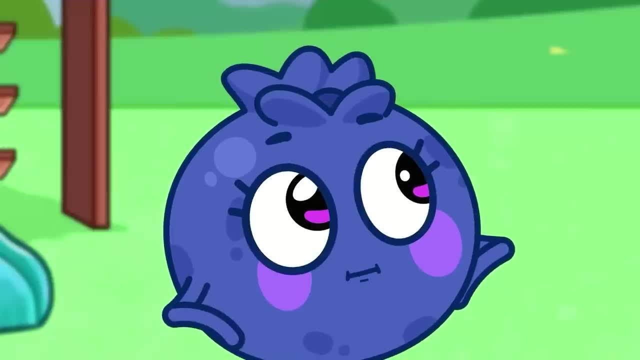 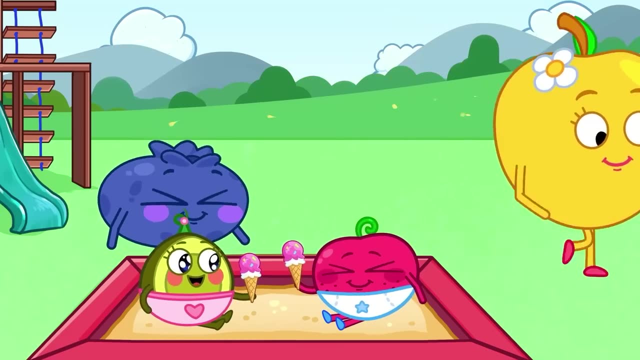 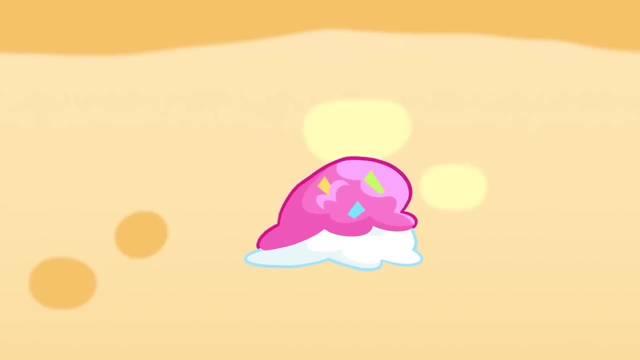 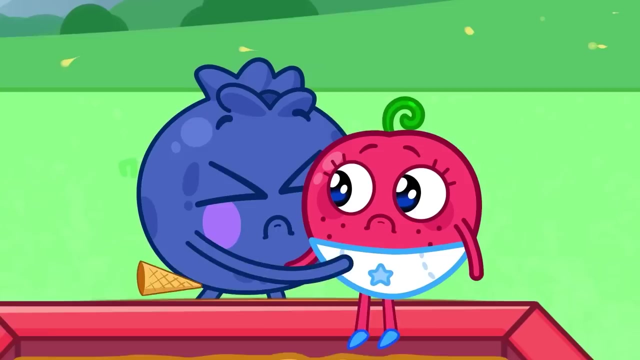 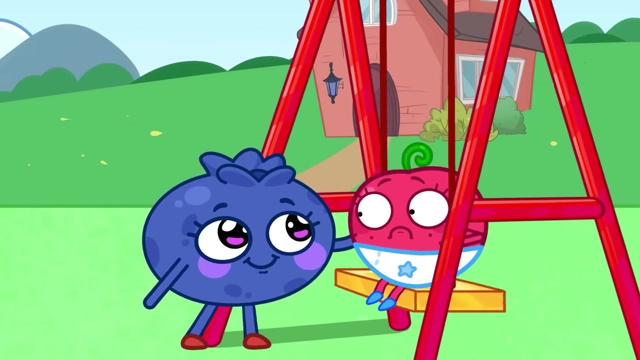 Who is it? It's not easy. I can handle two babies. It's a lot of work. Blueberry- Baby Cherry dropped her ice cream, But how can Blueberry stop Baby Cherry from crying? Yay, Baby Cherry loves playing on the swing. 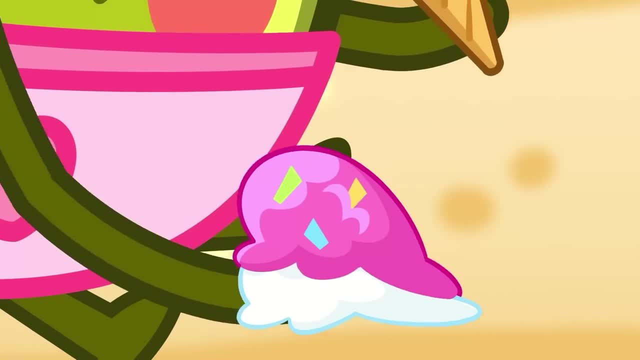 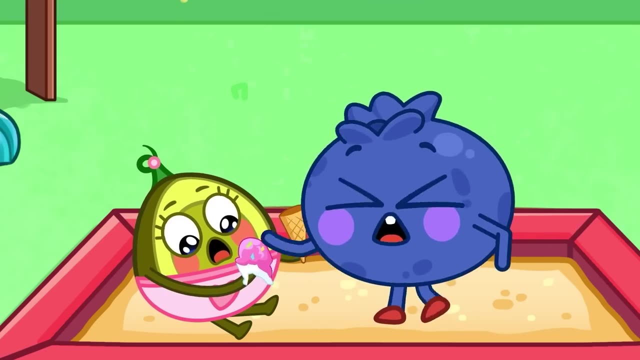 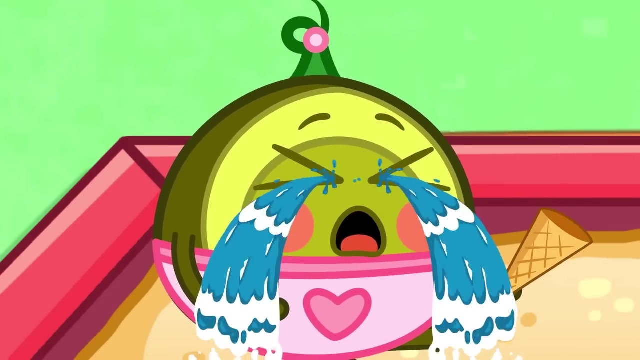 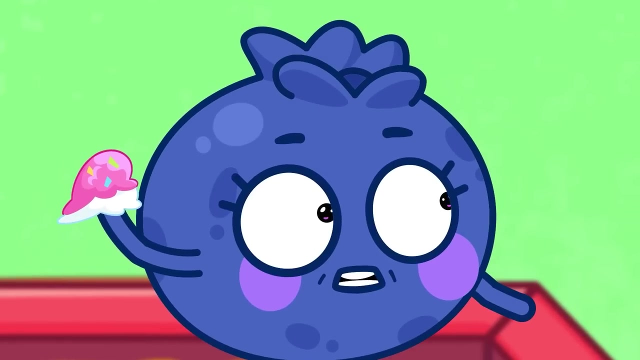 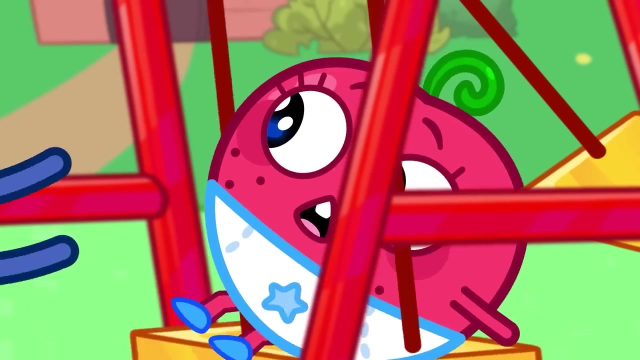 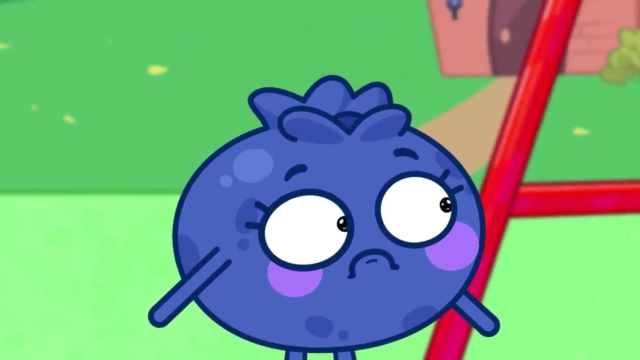 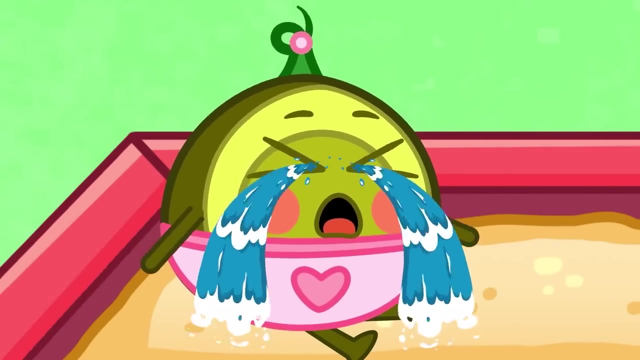 Now Baby Avocado dropped her ice cream. She still wants to eat it. You can't eat it. It's dirty. Now Baby Avocado's crying And Baby Cherry's about to fall. Blueberry saved him. Blueberry, Blueberry. 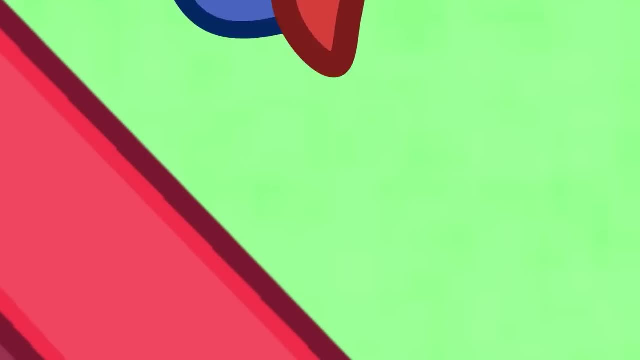 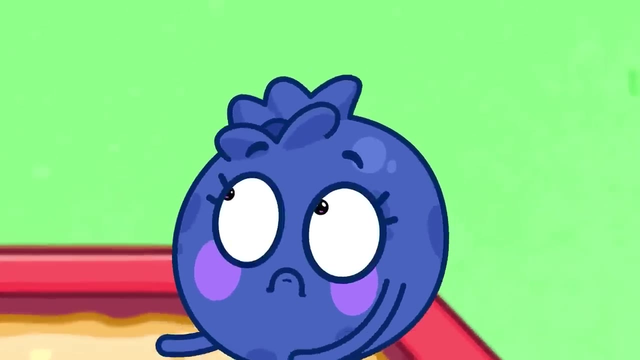 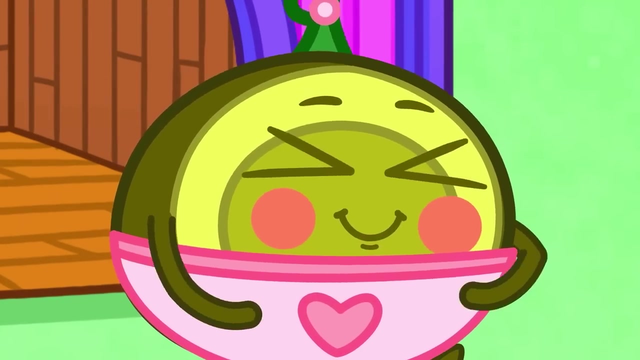 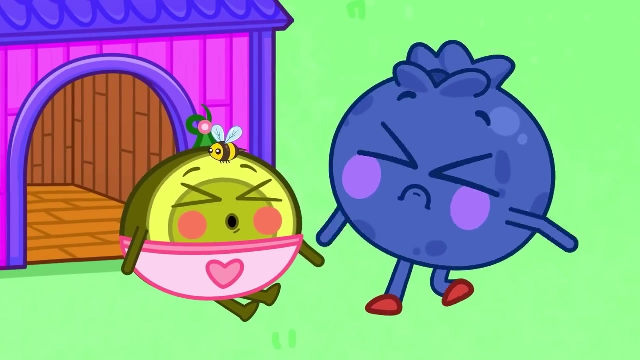 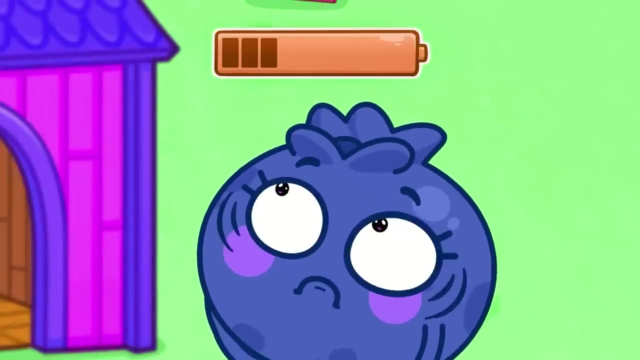 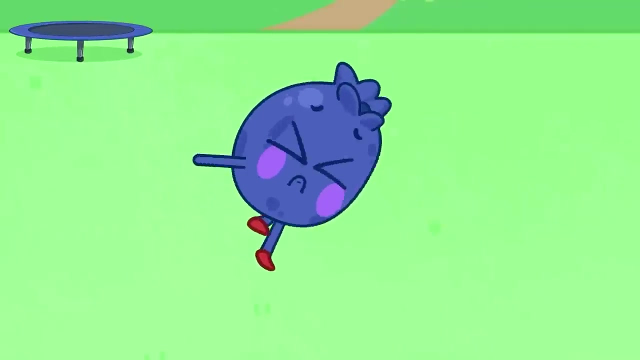 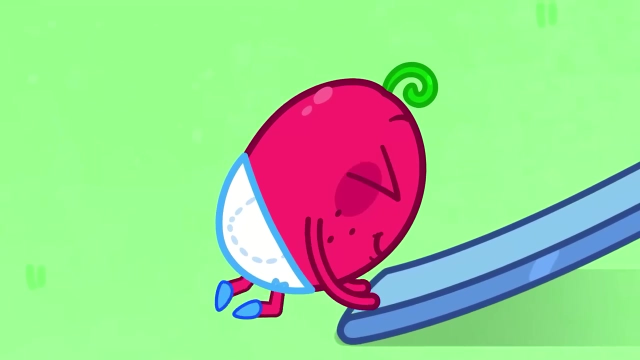 Don't forget about Baby Avocado. Oh, oh, oh oh. A bee is buzzing around. Baby Avocado, It might sting her Blueberry. shoot it away. Oh, oh, Oh. no, Where is Baby Cherry? He's climbing up the slide. 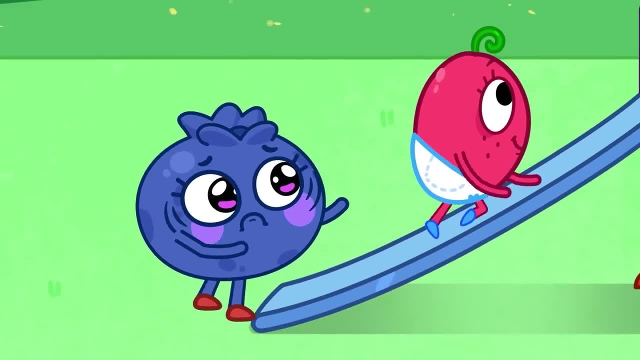 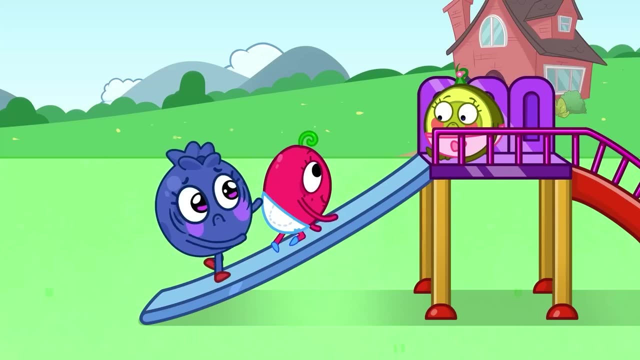 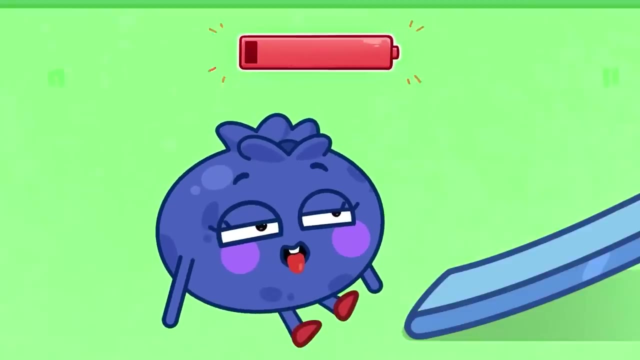 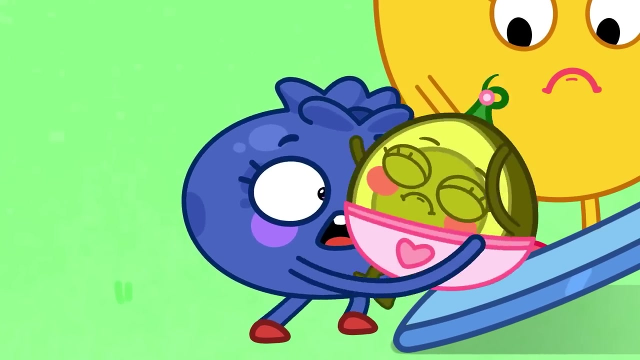 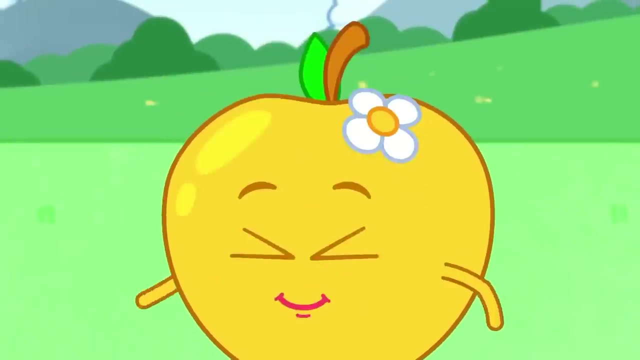 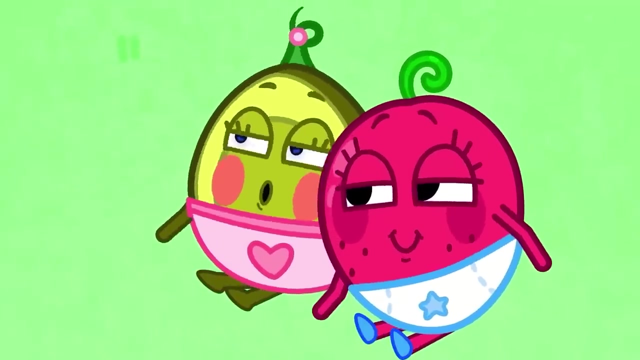 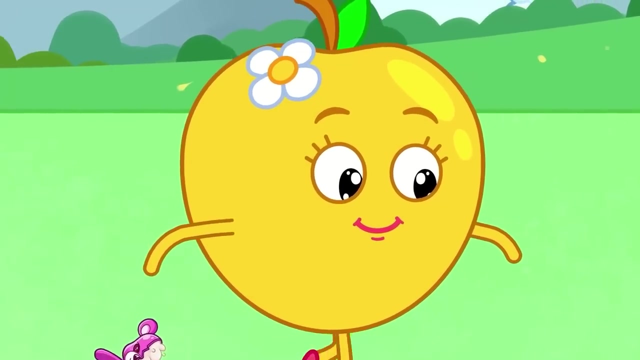 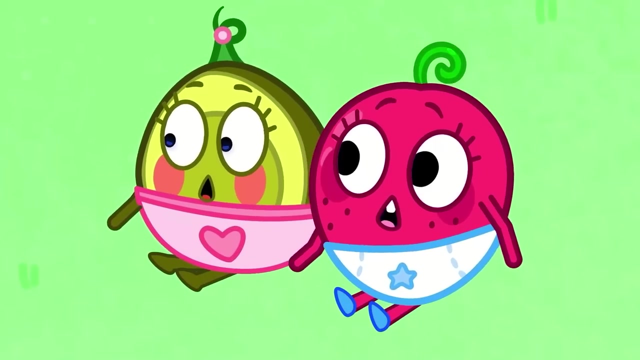 Taking care of two babies is a lot of work. Uh-oh, Baby Avocado will crash into Baby Cherry. Miss Apple arrived just in time. Caring is not only games. See, Everyone needs to rest. Watch out, That woke up the babies. 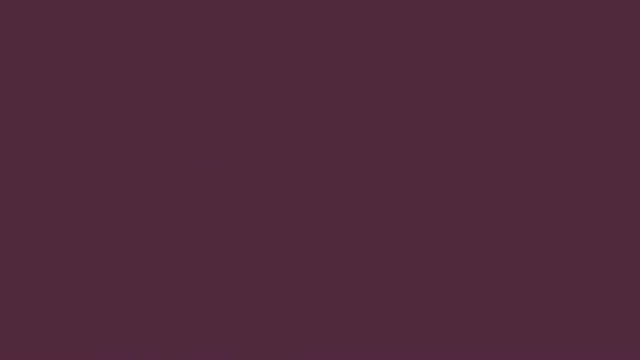 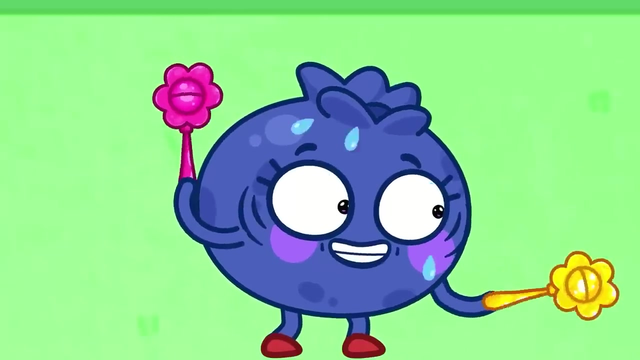 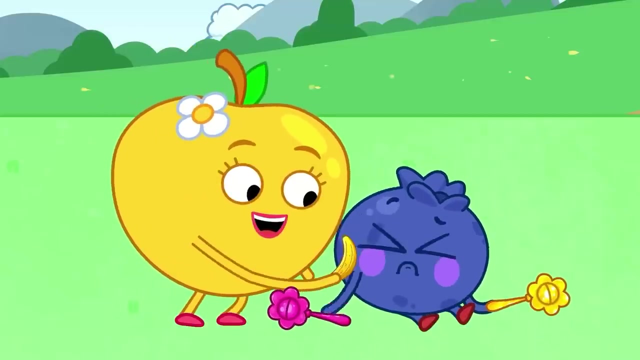 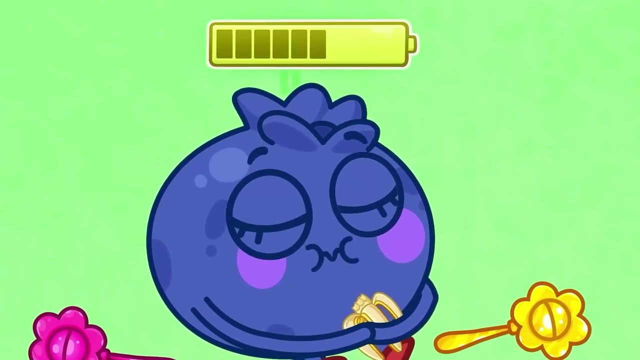 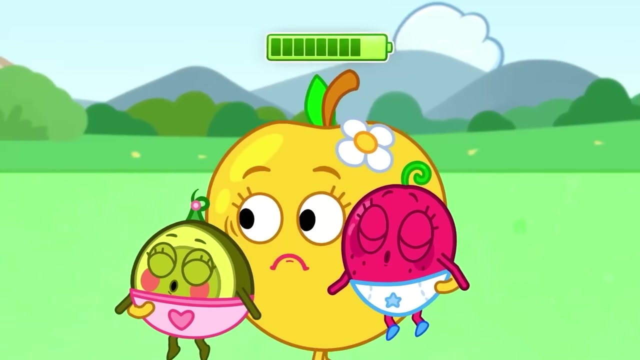 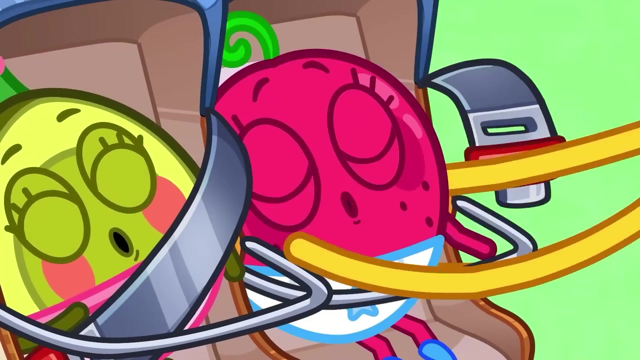 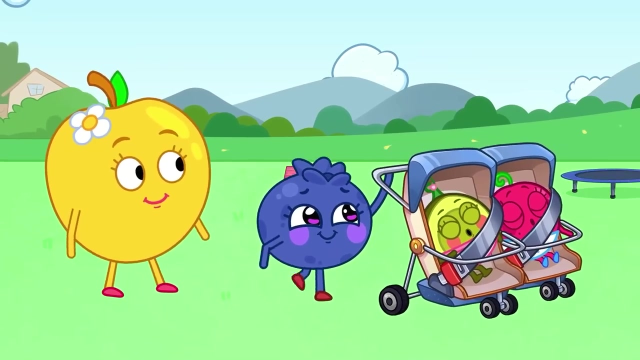 Blueberry will help them relax. Blueberry has no more energy. A snack will help It worked. Miss Apple is tired now and needs some help. You're a good babysitter. Well done. Blueberry, Kid and Penny have a new toy. 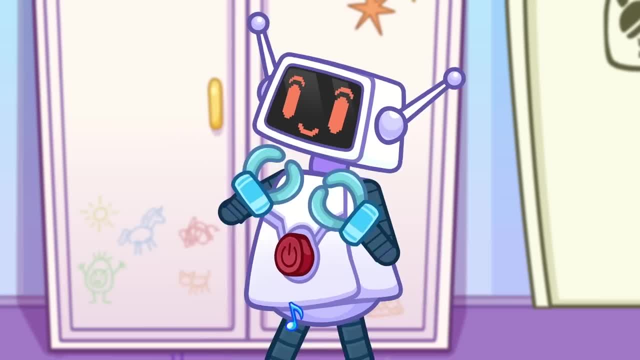 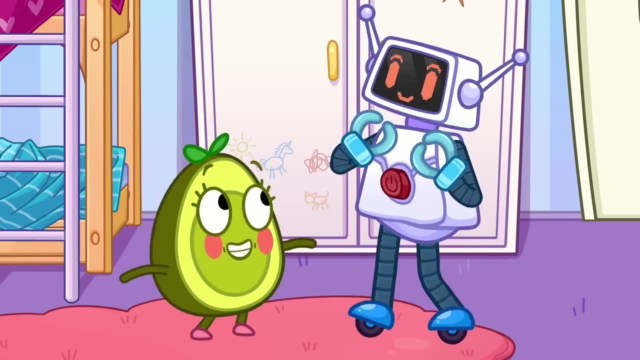 And it wants to teach them how to dance Clap Clap Cha-cha-cha. You try, Penny? Clap, Clap Cha-cha-cha, Clap, Clap Cha-cha-cha. 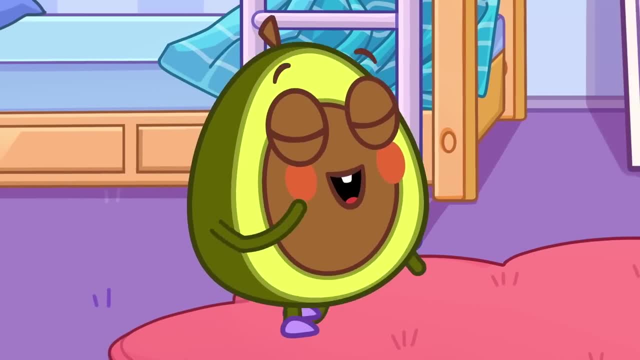 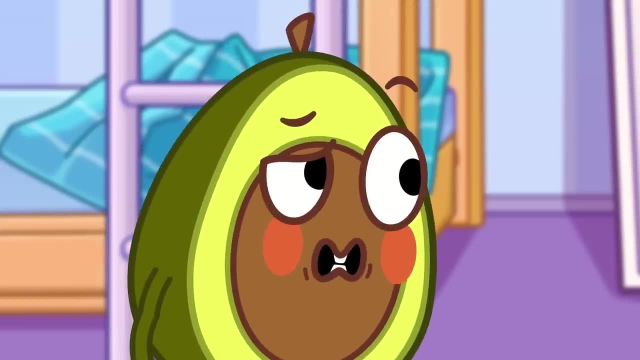 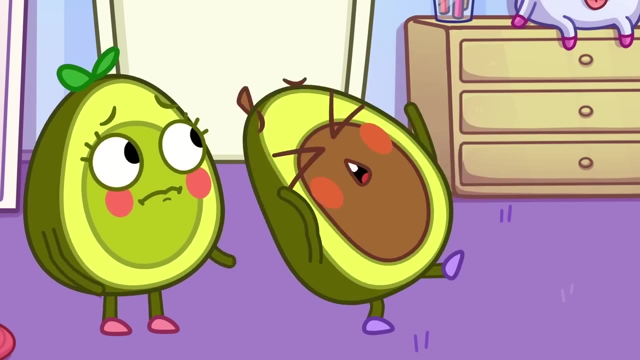 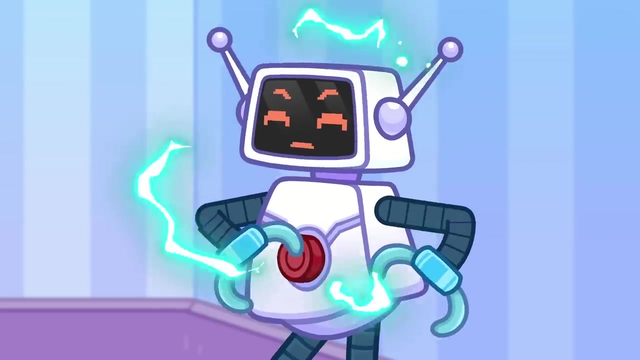 Your turn, Pit, Cha-cha-cha, Cha-cha-cha, Cha-cha-cha. Oops, Pit forgot to clap. Carefully, He's in pain. Look, Pit, You broke the robot. Clap, Clap, Cha-cha-cha. 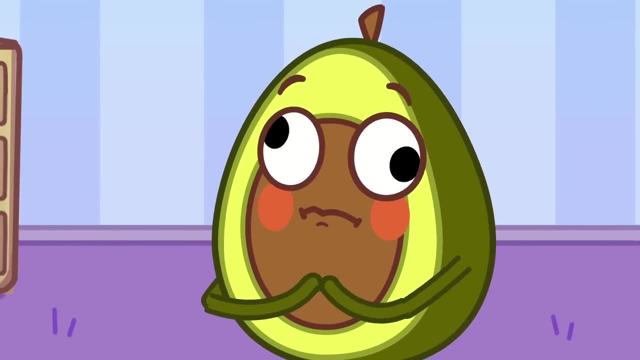 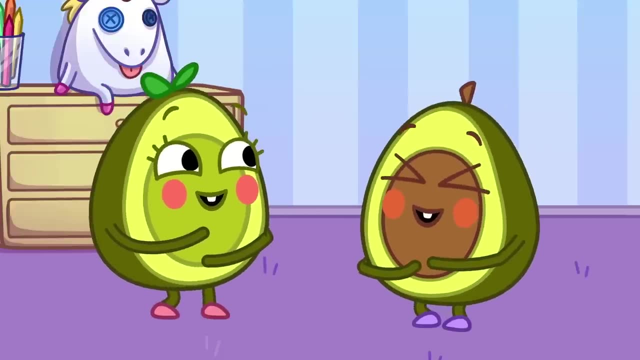 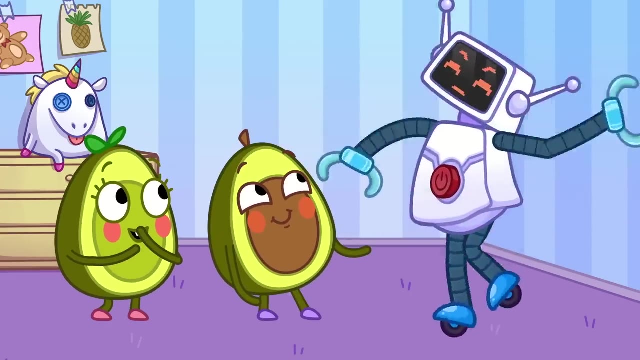 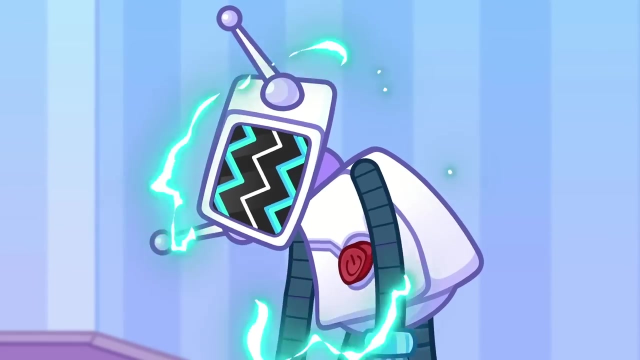 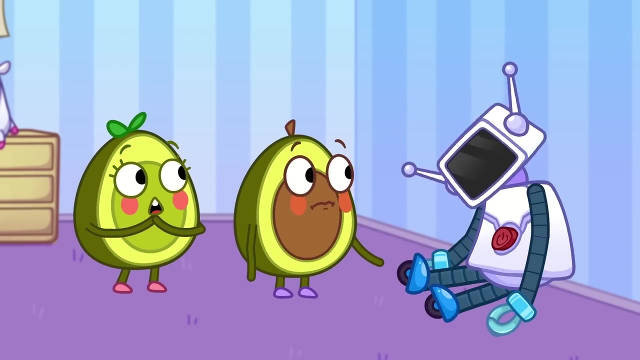 Clap, Clap, Cha-cha-cha, Cha-cha-cha. Pit thinks the robot sounds funny, And now faster. Oh no, Now the robot's really broken. Hey, Wake up. Oh, What have you done? 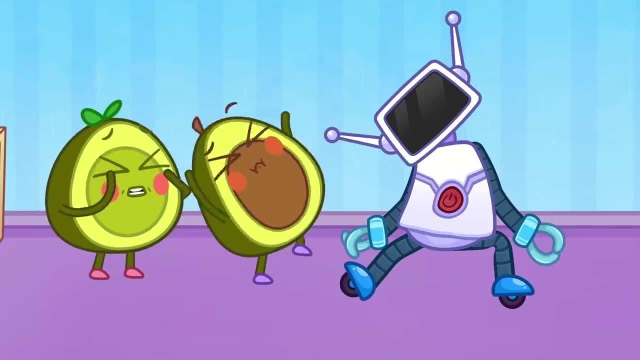 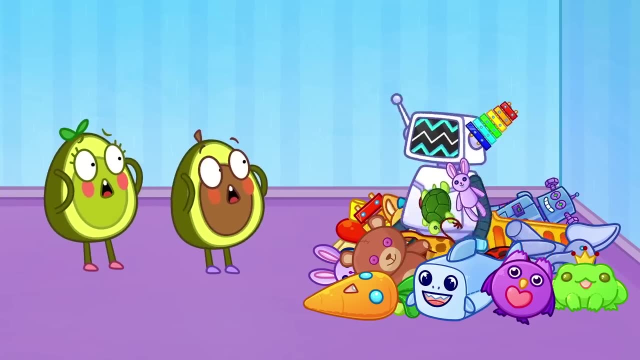 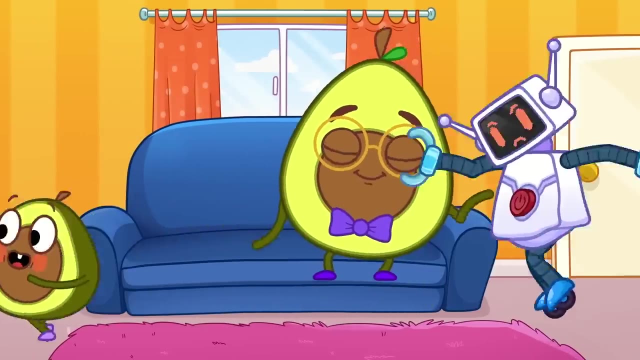 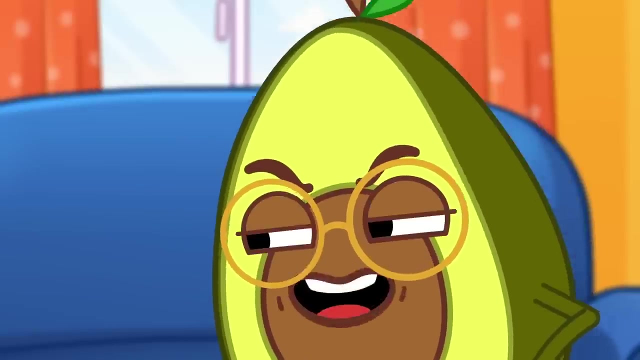 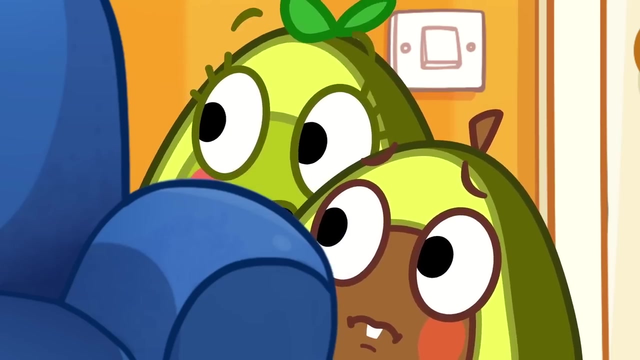 What a useless toy. Pit just wants to throw it away. What's this? Run The robot's out of control. Pit and Penny need Daddy's help. What's happened? kids? Oh yeah, Pi Grrr Ooh. 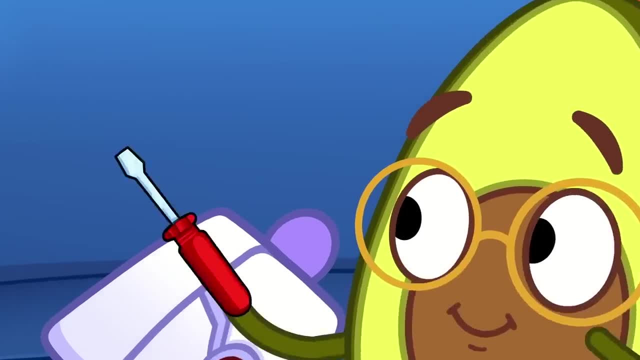 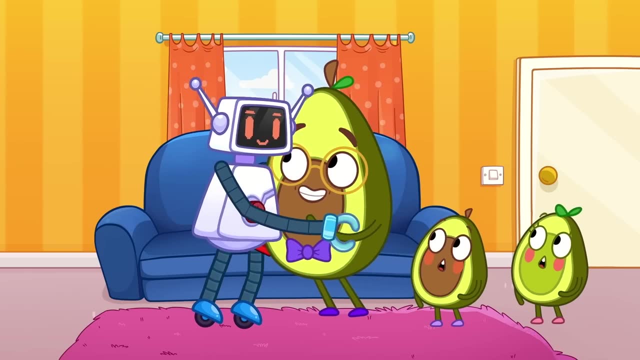 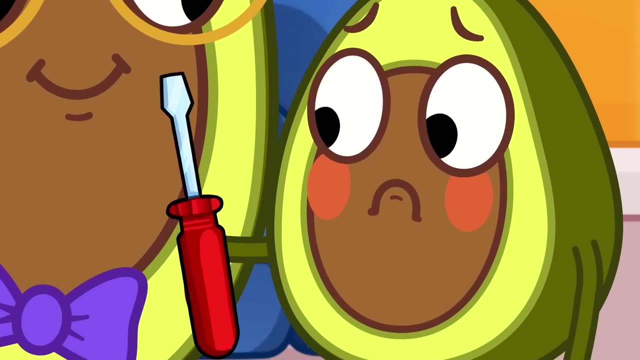 Looked like some help is needed. Daddy knows what to do So much better. The robot has improved. What a good little robot he is, Thank you. You should be careful with your toys. It's sad What's wrong, But I won that crazy dance again. 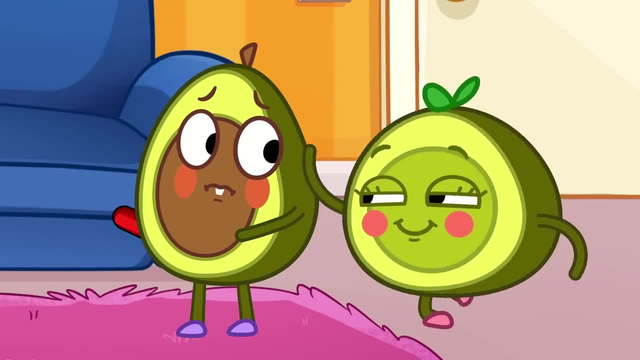 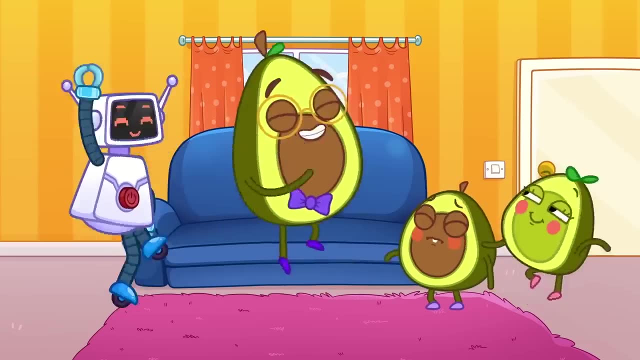 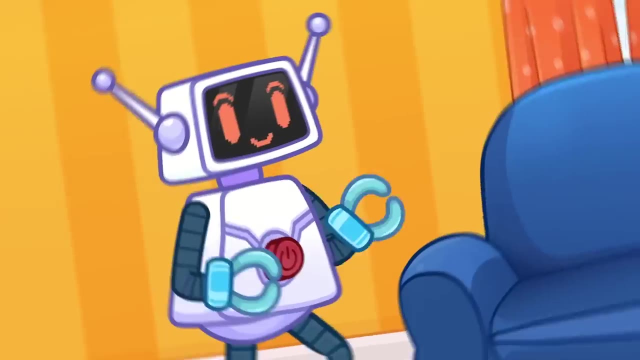 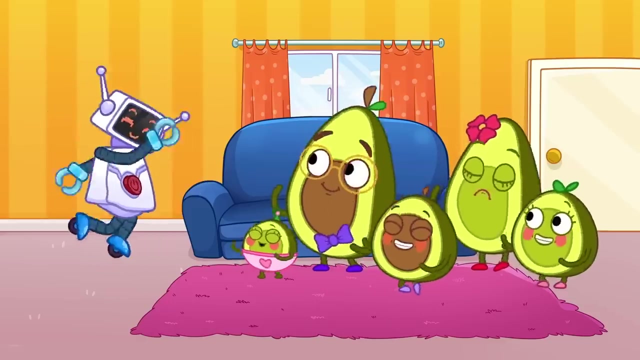 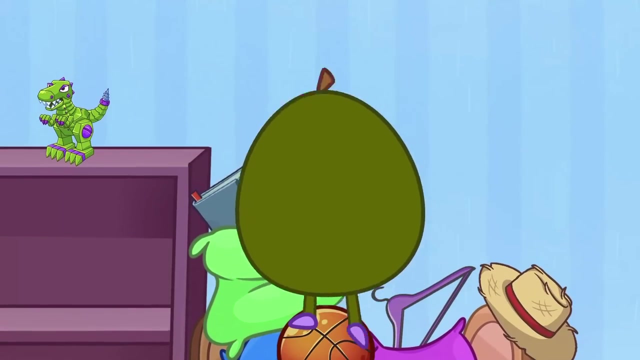 He's has been crying for too long. Dad, Rip it off to me. Just copy, Penny. I'll try too. Let's see Pit do it Now. everyone can dance together. Don't climb up there, Pit, It isn't safe. 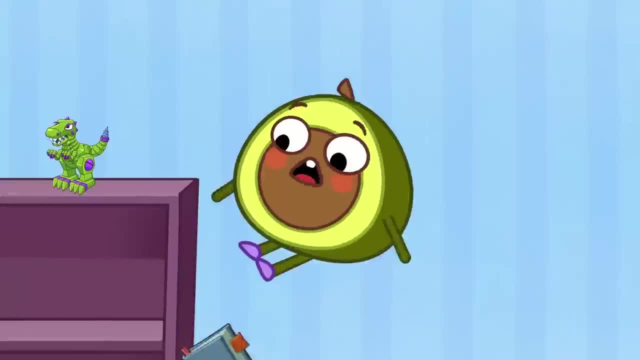 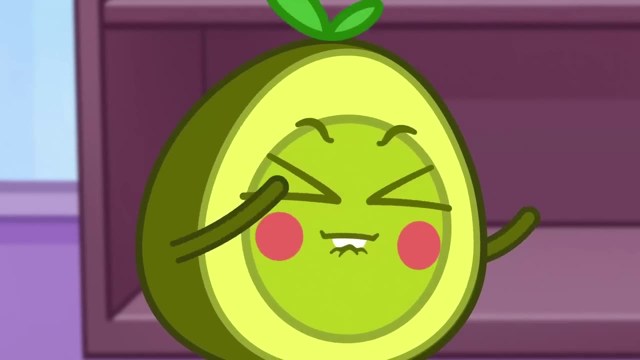 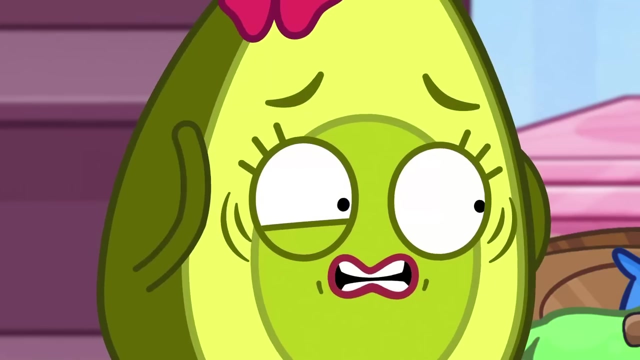 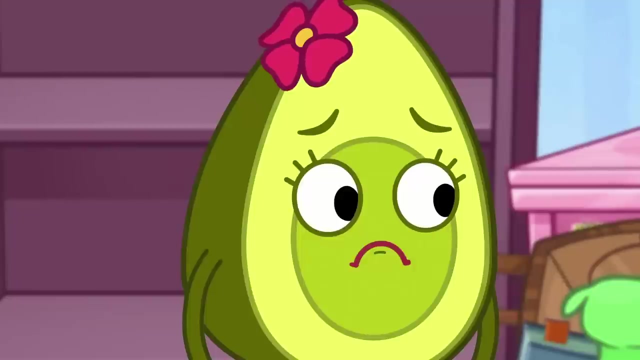 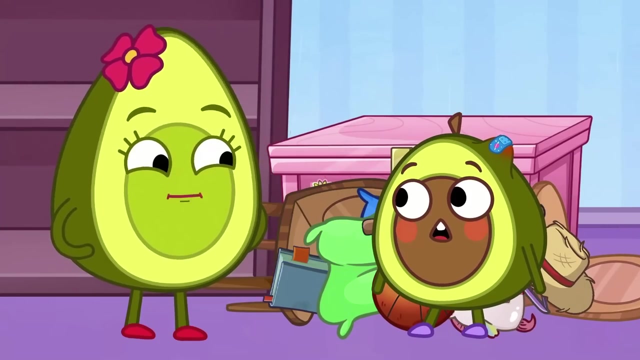 Penny, Help me. Pit had an accident, I'll save you. He bumped his head in the fall. Mommy knows what to do. Oh, Kiss, If something happens, call your parents. What should you do if you can't reach a toy? 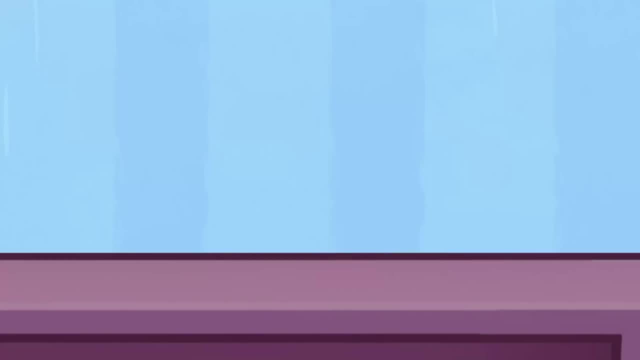 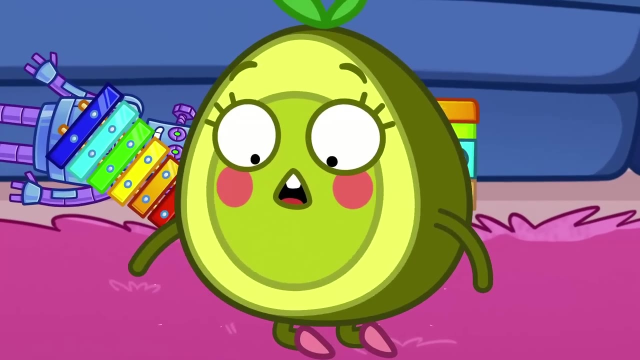 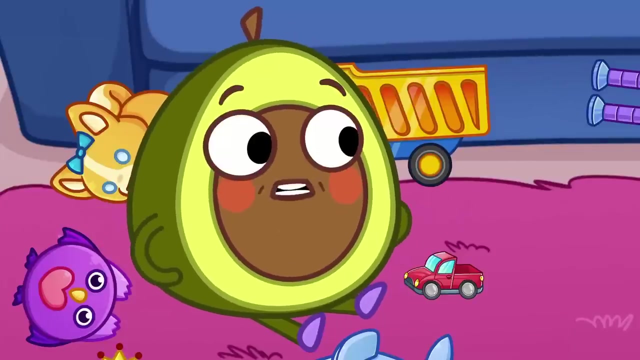 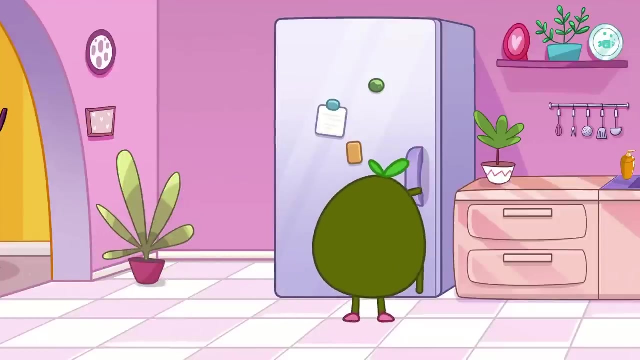 Ask parents for help. That way you won't get hurt Penny's hungry. Wait, Penny, What about your mess? Can we pick up the toys together first? Let's go, Penny, Wait, we can't give up. Is a toy not enough? 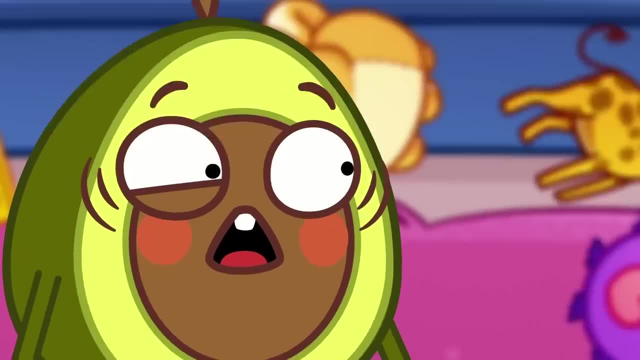 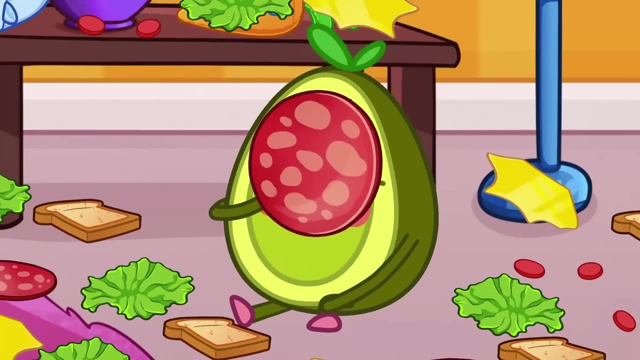 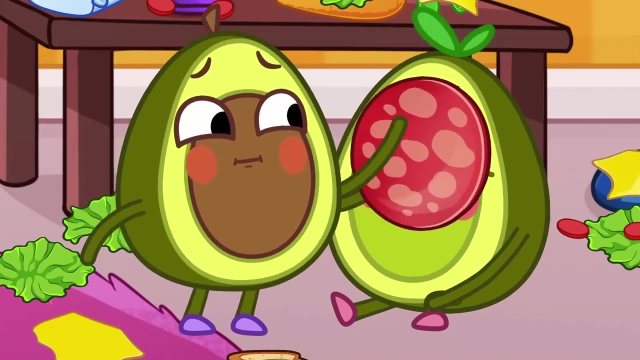 Yeah, What's wrong? Pit Penny is going to trip. What should you do? Pit Penny's hurt. She needs help. Penny's breathing is getting worse. She's going to tripple. Penny is going to tripple. 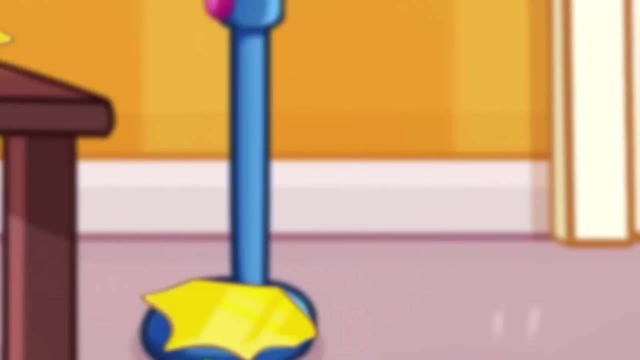 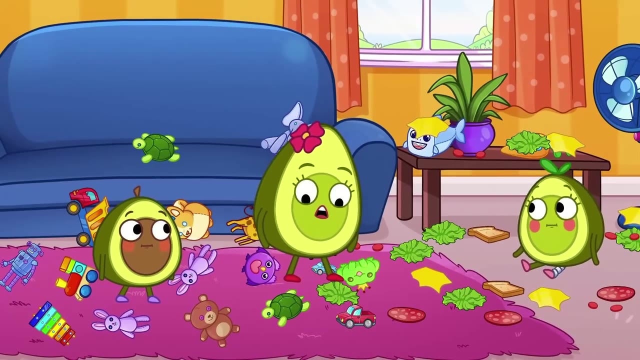 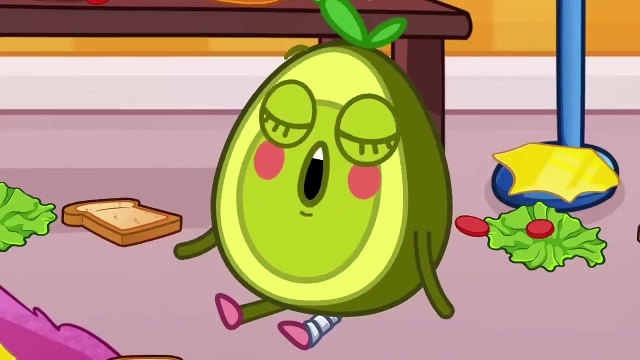 You can't move, You can't move, You're not going anywhere. No, No, No, No. And mommy made it better. What do you have to do to avoid injury? Pick up the toys Now. there's nothing to trip on. 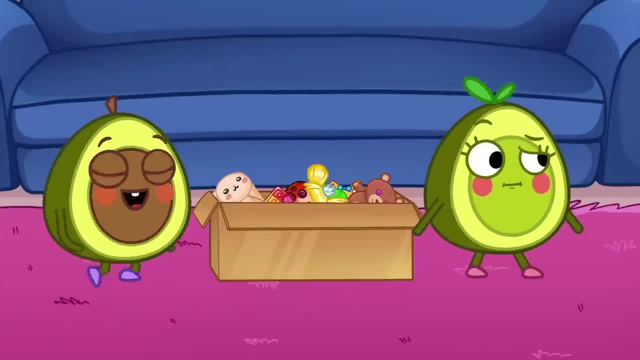 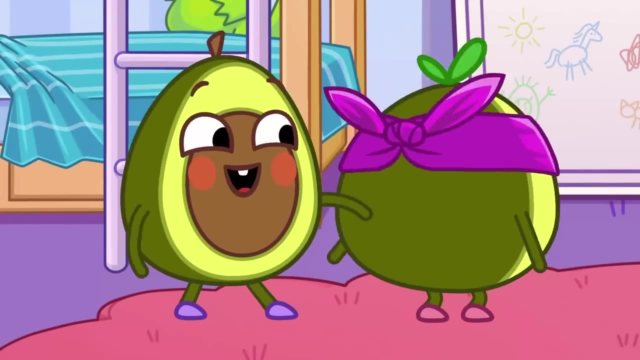 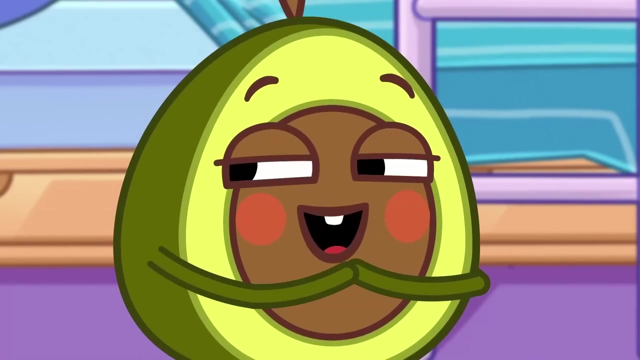 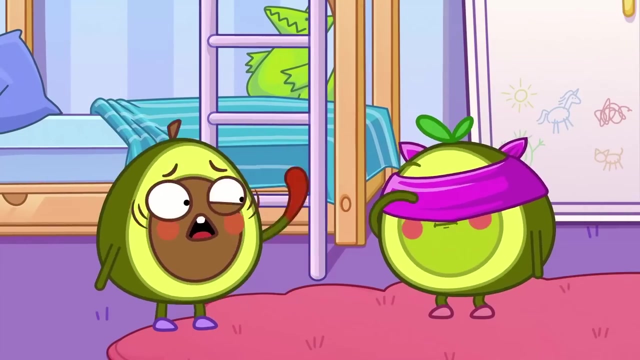 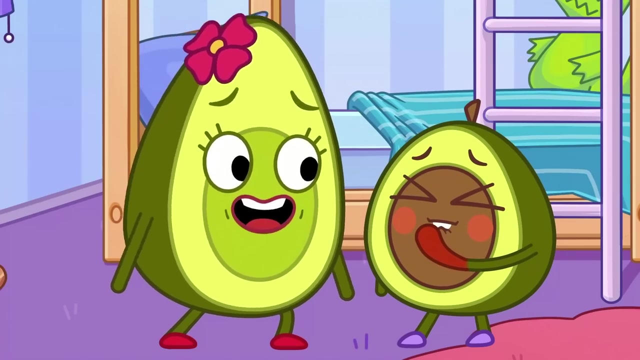 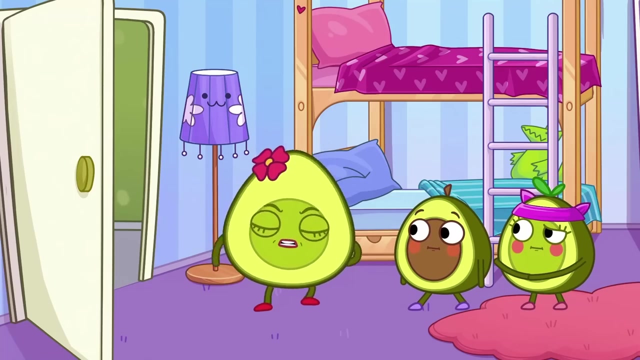 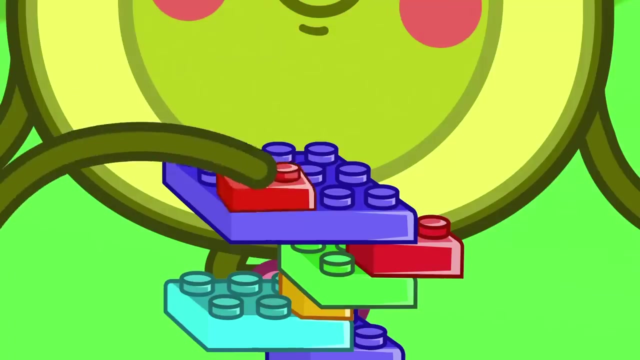 Let's play hide-and-seek. You can't hide from me. You can't catch me. Oh no, Pit's arm got caught in the door. Mommy will make it better. Pit, don't use doors in your games. That toy looks like candy to Baby. 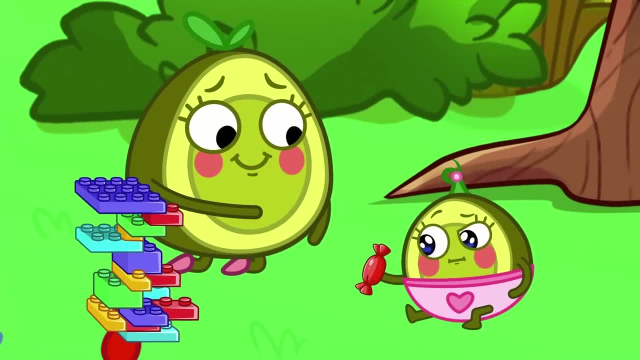 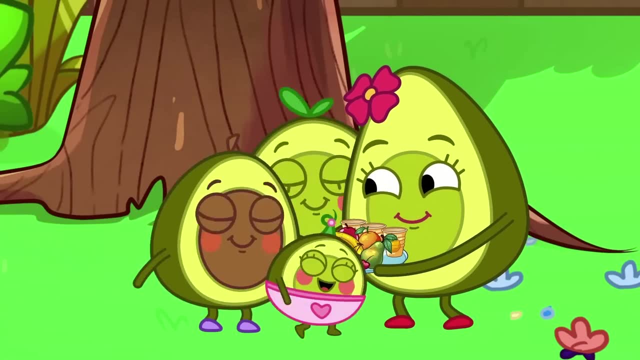 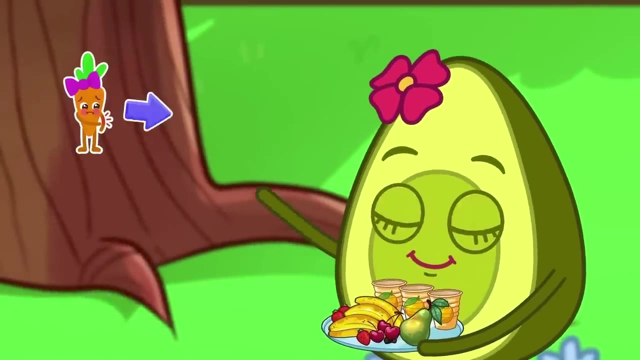 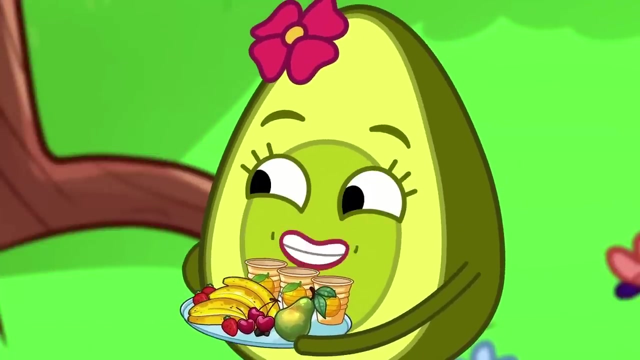 No, You can't eat toys, Right, but what can you do? I don't know how to eat. Do you know, Pit? Help me, Boo. In case of an accident, always call your parents. They'll keep you healthy and safe. 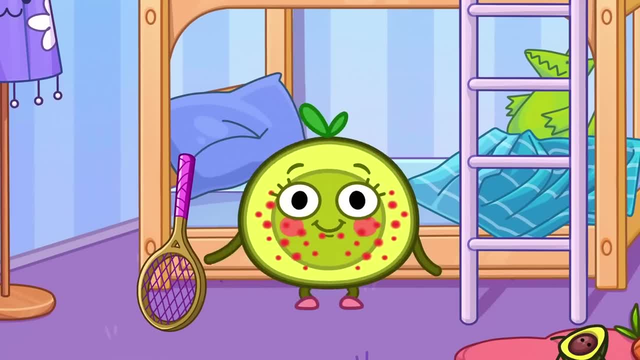 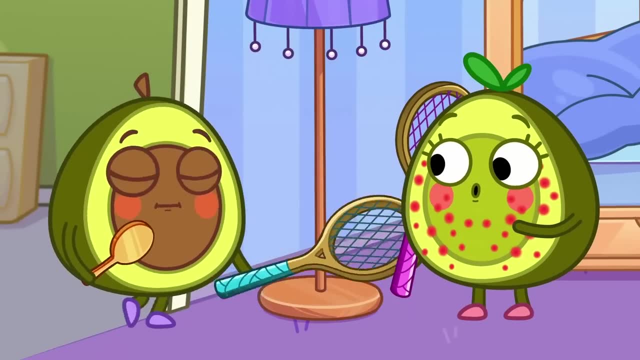 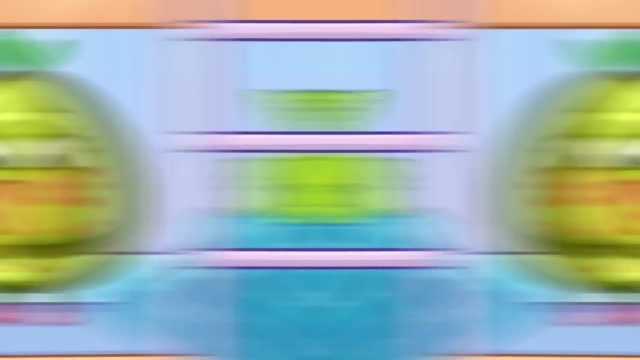 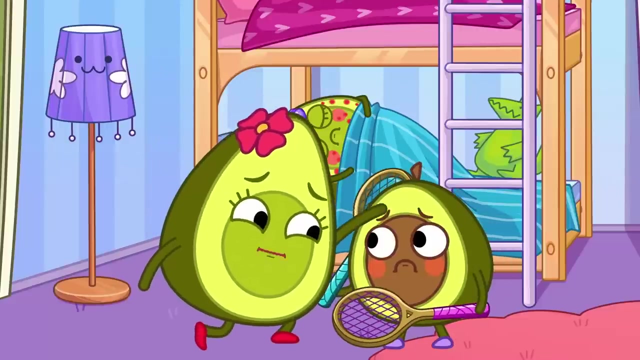 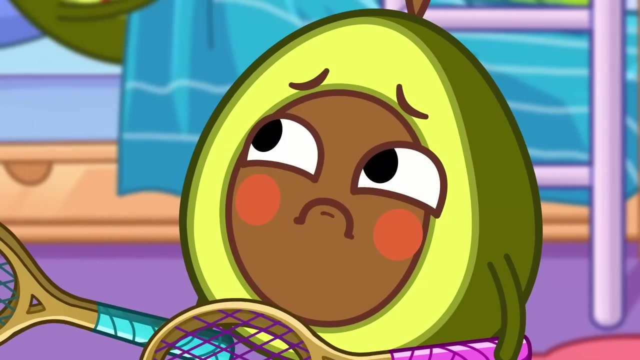 Hey, Penny, How about a duel? Okay, Pit, Look, Penny, You're covered in spots. See for yourself, It's chicken pox. Can we still play? No games, Pit, Your sister is sick. Okay, Mommy, Now what will I do? 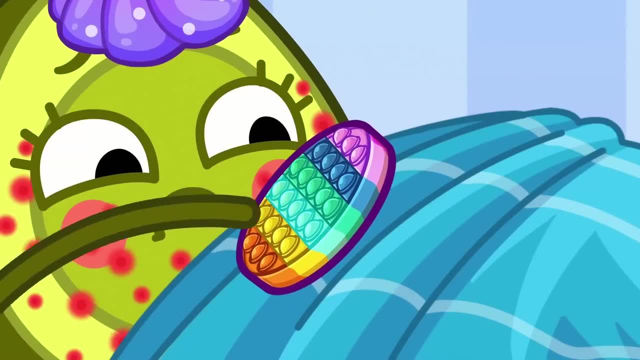 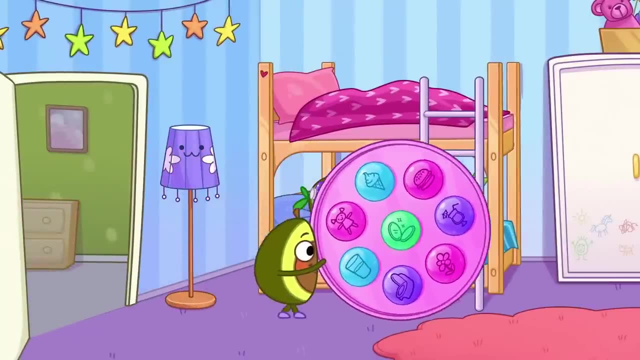 I can't do anything. I can't do anything. I can't do anything But play, pop it. I know what to do. Coming through, What's this Pit? Look Here, Point out what you need and I'll get it. 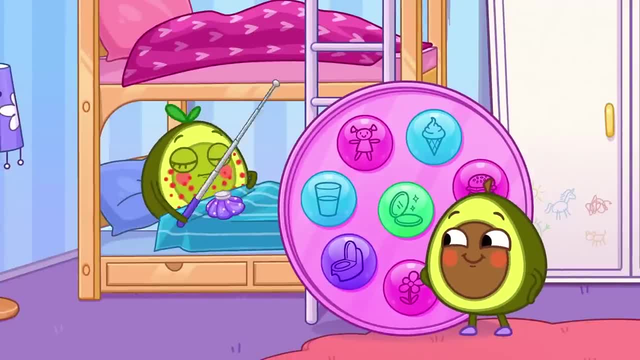 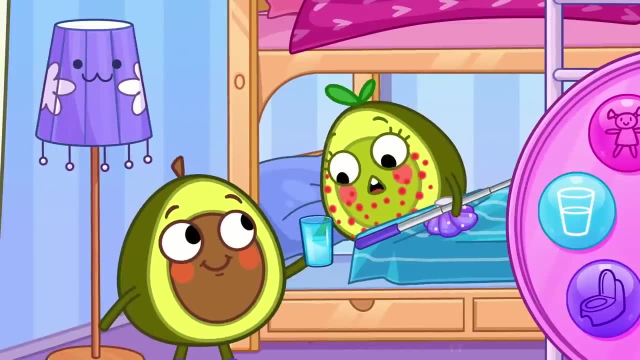 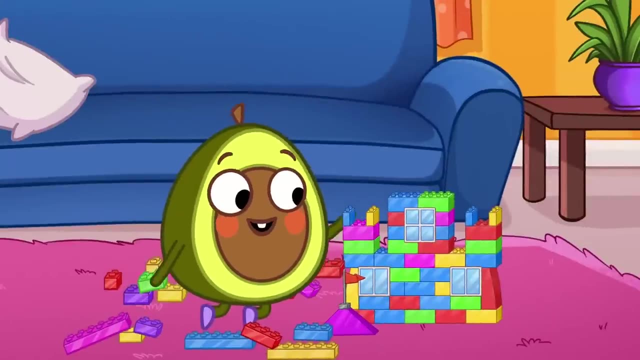 Here. Point out what you need and I'll get it. A glass of water, please. A glass of water, please, Coming right up, Here you go, Here you go. Thank you, Pit. Thank you, Pit. This will be my biggest castle yet. 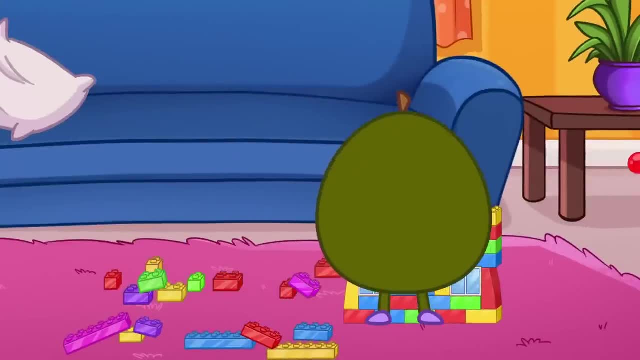 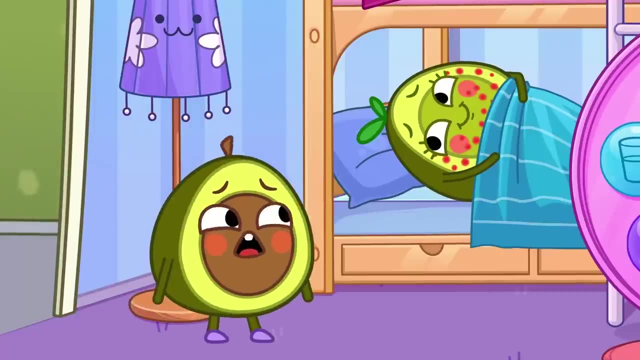 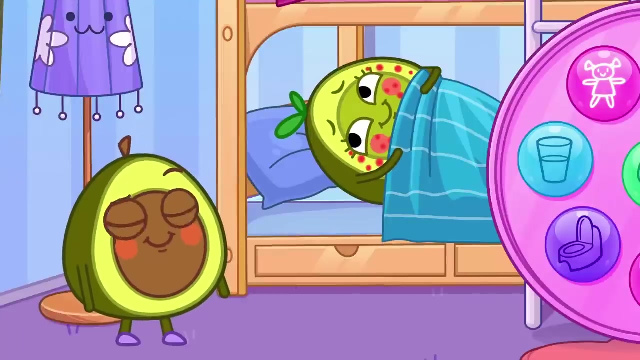 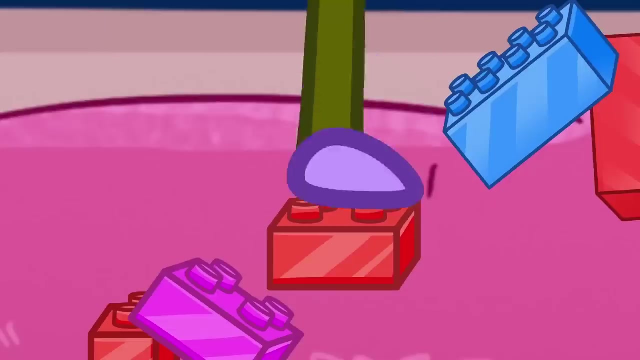 This will be my biggest castle. yet. One last piece. One last piece. What was that? Penny needs me. I need my doll. Please Be right back. It must be right over here. It must be right over here. That really hurts. 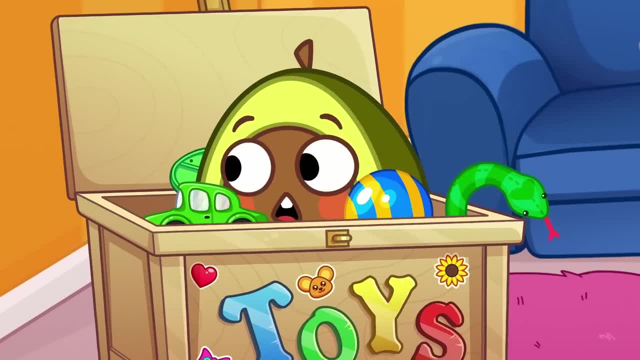 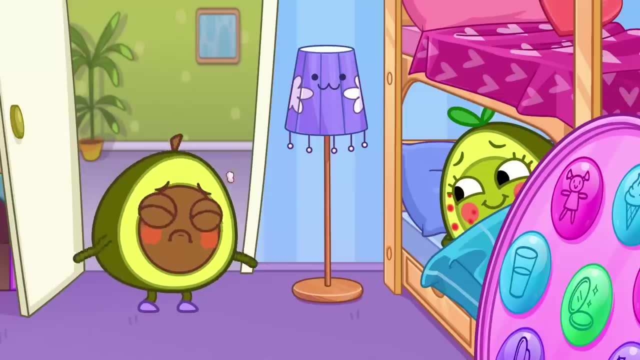 Ow, Ow, Ow Ow. I bet the doll is in here. I bet the doll is in here. I bet the doll is in here. I couldn't find your doll. I couldn't find your doll. Sorry, Here she is. 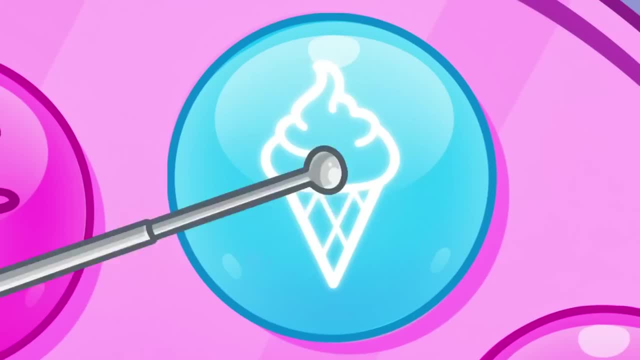 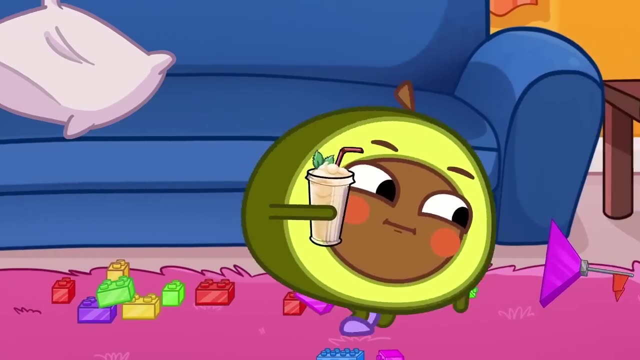 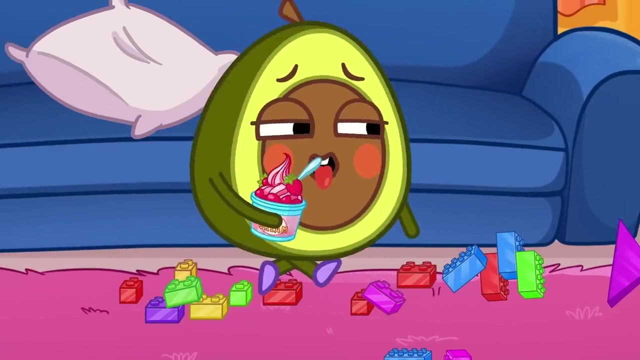 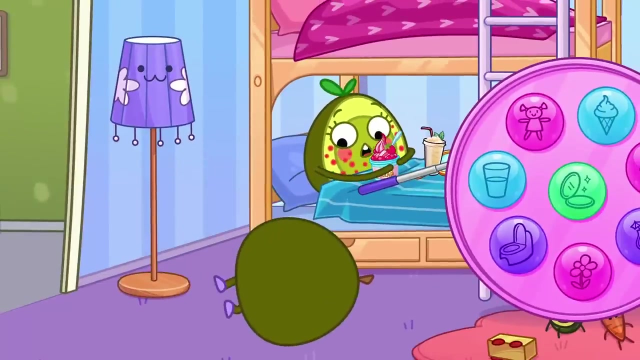 That's not very funny. Penny, I need food And ice cream. I'll get it. Food, A drink, A drink Water And ice cream And ice cream Here. I'm tired. Flowers, please Come on. 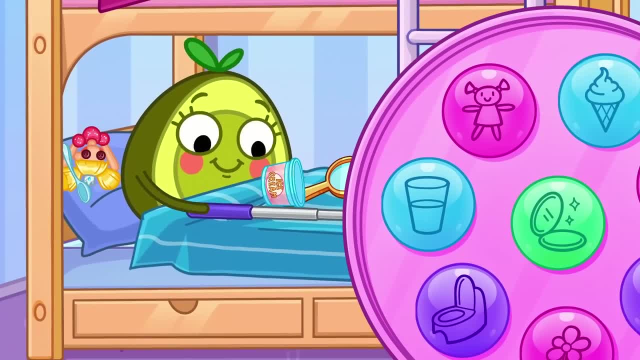 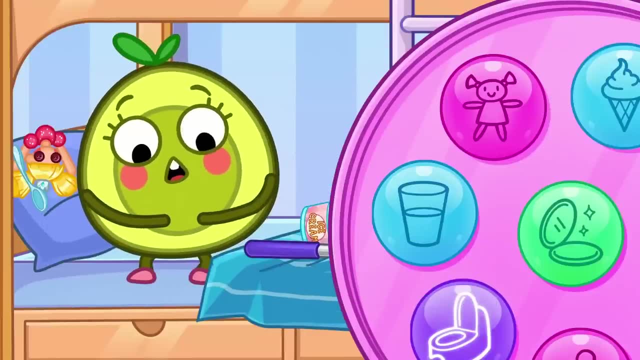 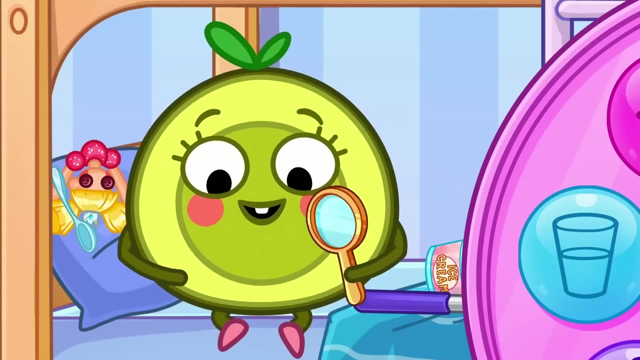 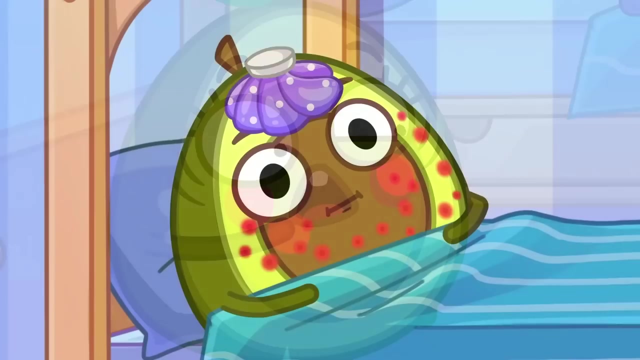 Okay, Now it's time for the potty. Pit, Pit, Where is he? He's sleeping. I'm not sick anymore. I'm not sick anymore. Pit, I can play now. Pit, I can play now. Now, he's sick. 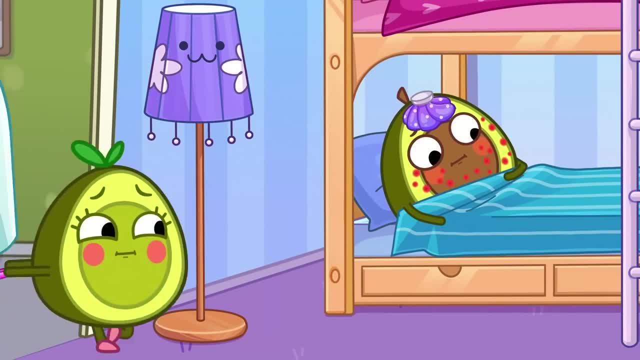 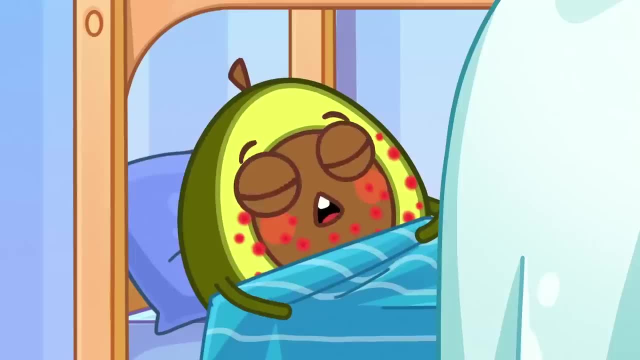 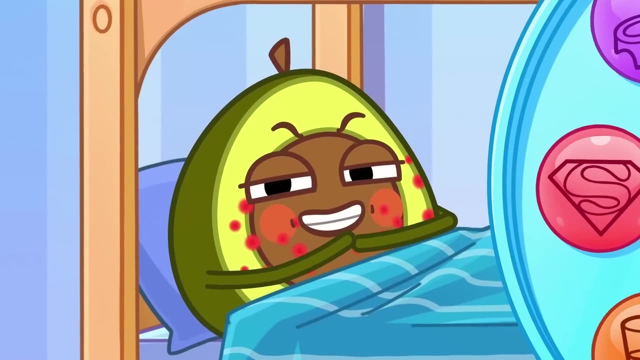 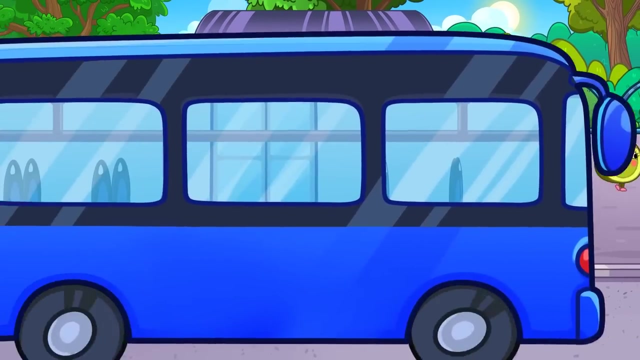 Now he's sick. This is for you, because I'm sorry for my behavior. What is it Now? I help you. Ta-da, Ha-ha-ha. Pit and Penny are waiting for the bus. Oh look, Here comes the bus now. 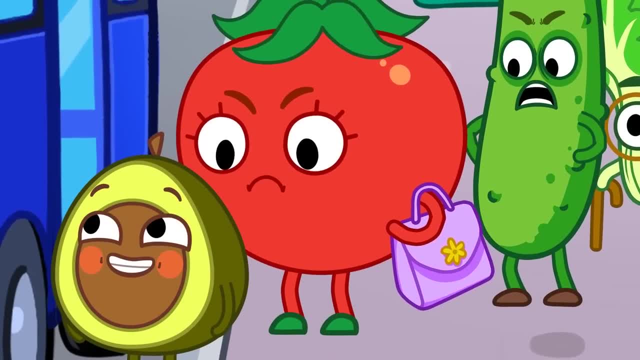 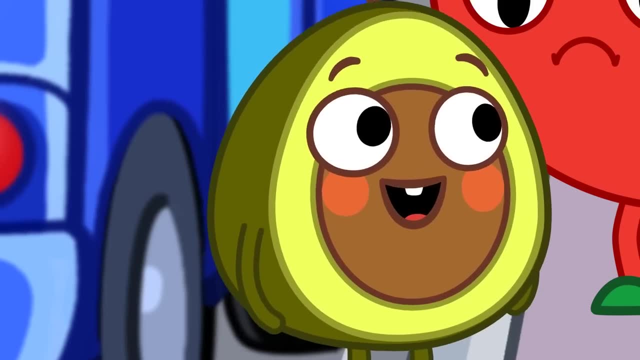 Pit butts in front of everyone. Miss Tomato isn't very happy. Miss Tomato isn't very happy. Oh, Pit, you should stay in line. Uh-huh, uh-huh. It is always best to wait your turn. It is always best to wait your turn. 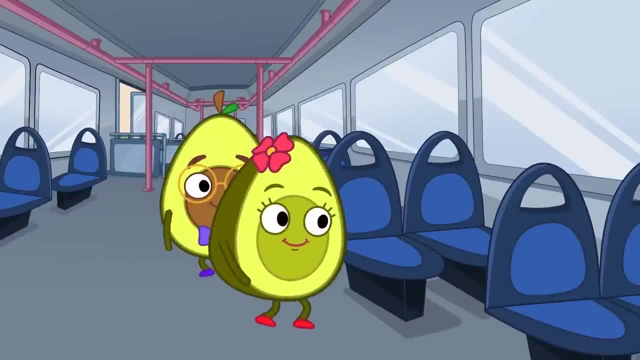 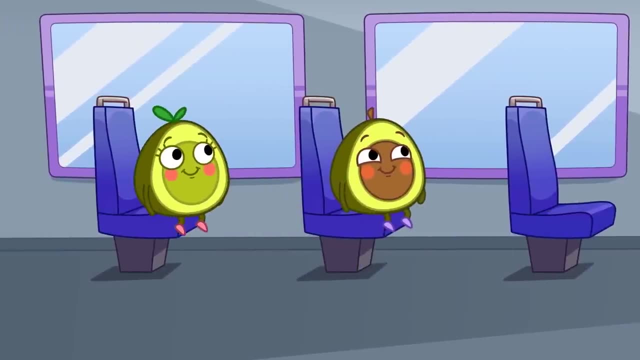 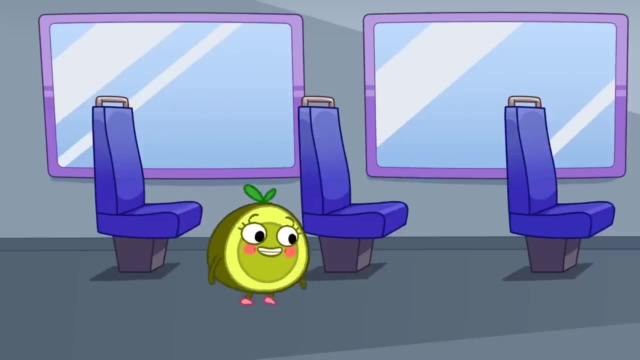 There are lots of places to sit. There are lots of places to sit. Pit thinks they should play a game. Pit thinks they should play a game. Penny wants to play too. Penny wants to play too. But you should always stay in your seat on the bus. 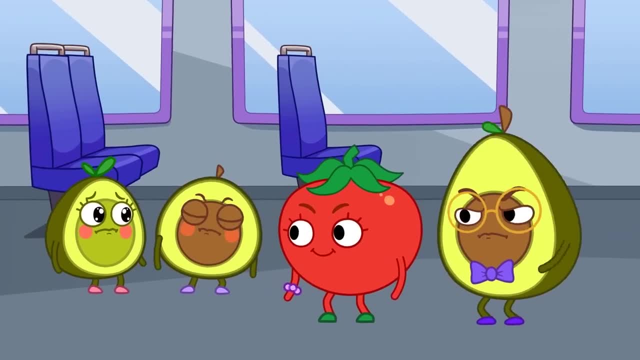 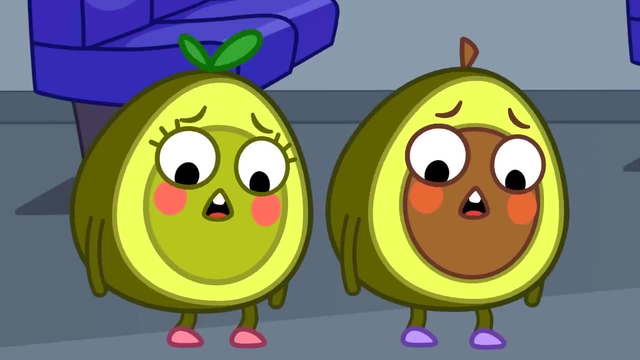 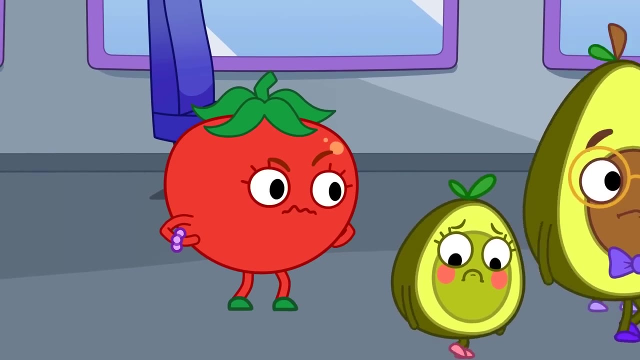 Or you could get hurt. Thank you, Miss Tomato. Thank you, Miss Tomato, But don't run in a bus. It's not safe. Okay, Okay, Okay, Okay, Okay. Now, more people are getting on the bus. Now, more people are getting on the bus. 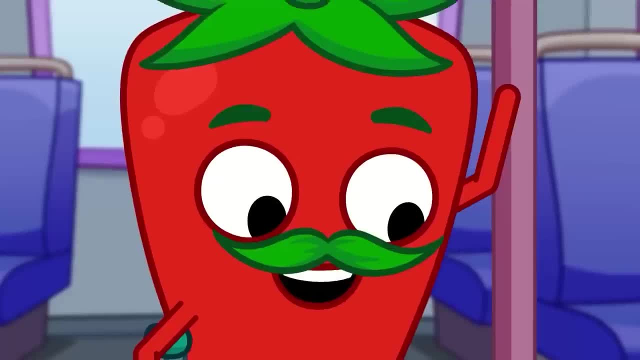 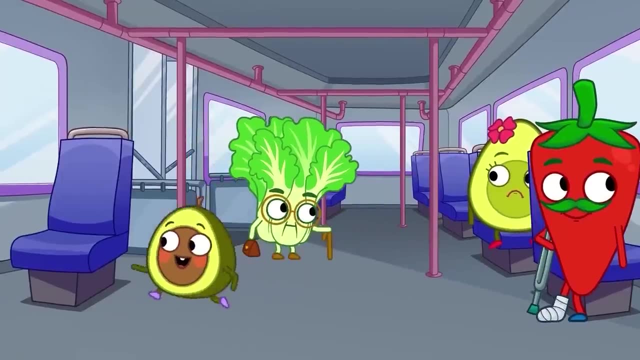 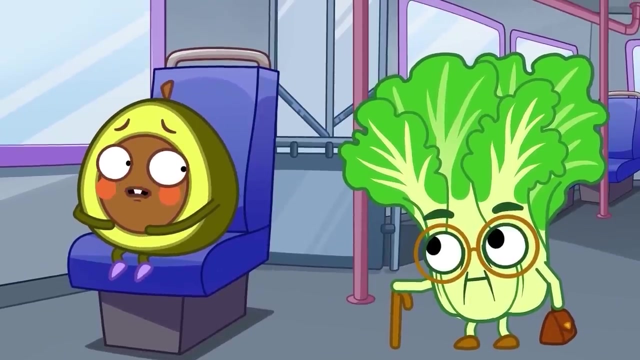 That man has a broken leg. That man has a broken leg. Thank you, young man. Well done Pit. Well done Pit. Well done Pit Pit. someone else needs a seat, Pit Whoops, I'm sorry. 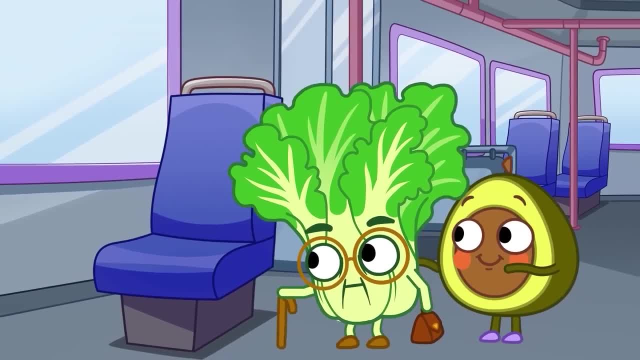 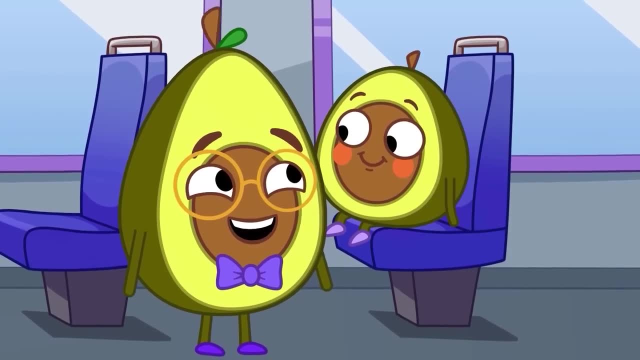 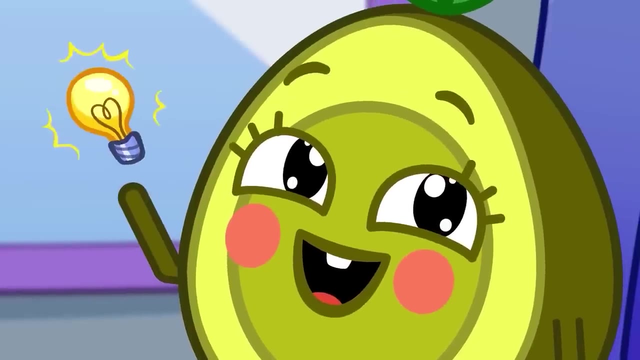 Whoops, I'm sorry. Here you go, Mrs Lettuce. Here you go, Mrs Lettuce. Here you go, Mrs Lettuce. Hmm, Ha-ha, Ha-ha, Shhh, Mrs Lettuce is sleeping. 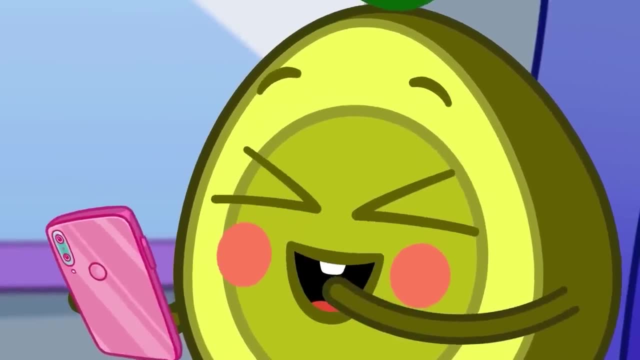 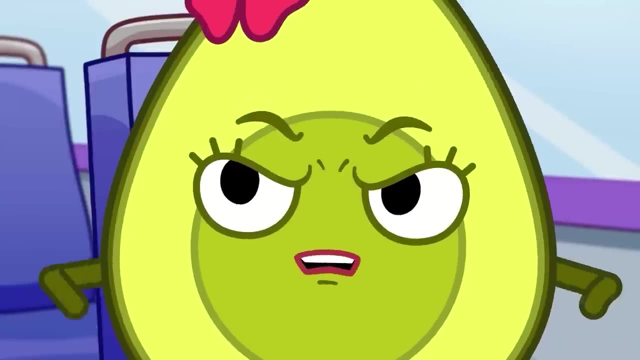 Mrs Lettuce is sleeping. Penny wants to watch some funny videos. Mrs Lettuce is sleeping, But the noise has woken up, Mrs Lettuce. But the noise has woken up, Mrs Lettuce. Penny, it's too loud. 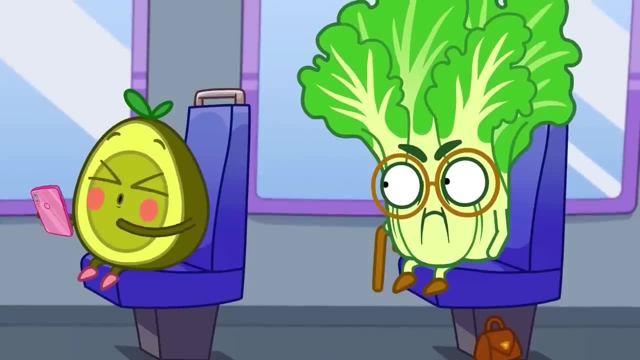 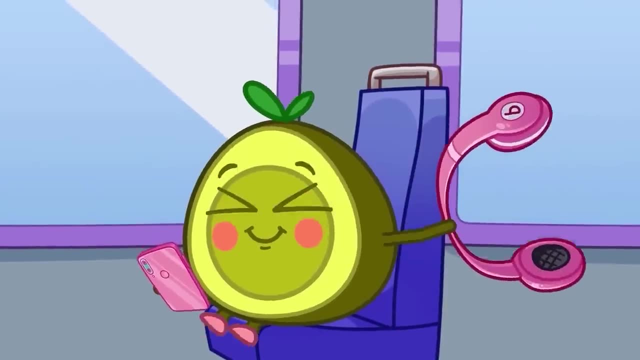 You'll disturb other passengers. You'll disturb other passengers. Okay, I'm sorry. Okay, I'm sorry, Penny, just use your earphones. Penny, just use your earphones. Ah, peace and quiet. Have a nice nap, Mrs Lettuce. 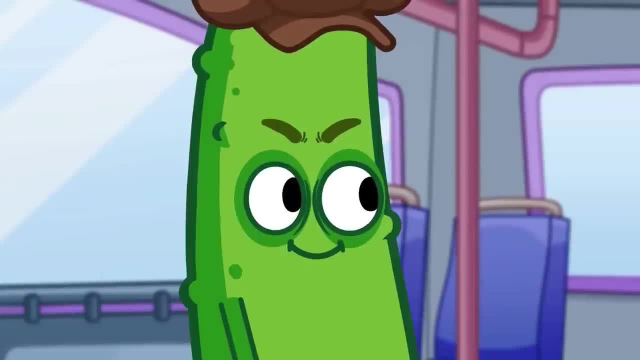 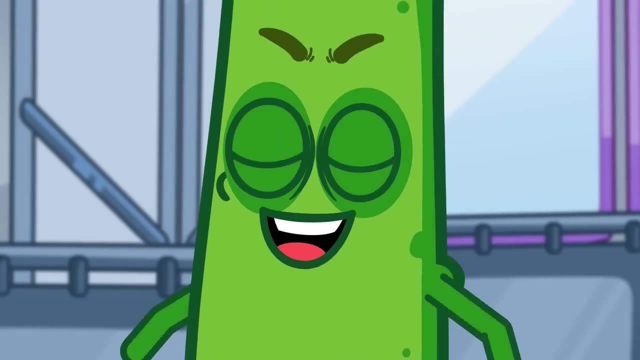 Have a nice nap, Mrs Lettuce. Hmm, This passenger looks suspicious. This passenger looks suspicious. Oh no, Mrs Lettuce left her purse on the floor. Mrs Lettuce left her purse on the floor. Someone should stop him. 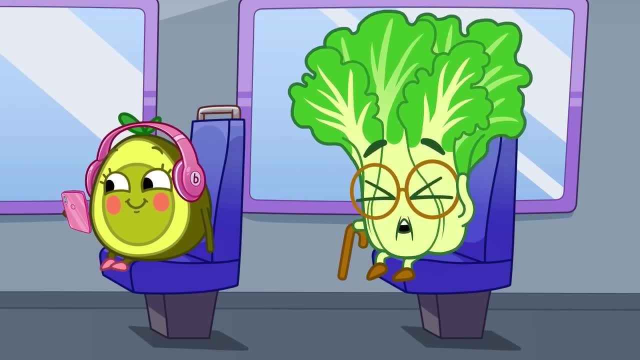 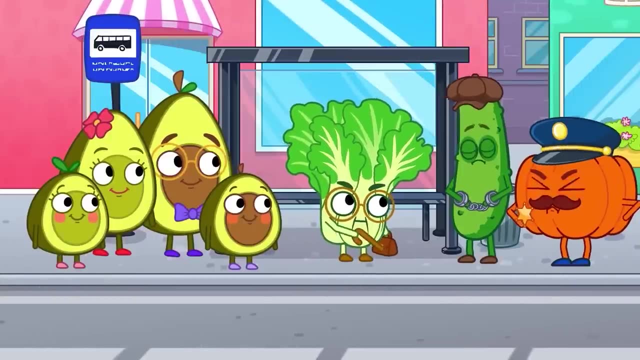 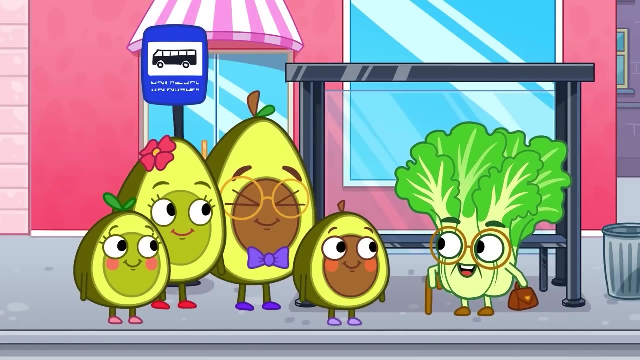 Someone should stop him. Someone should stop him. He's a thief. Pit has saved the day. Pit has saved the day. Thank you, young man. Thank you, young man, Well done. son Penny loves swimming in the ocean. 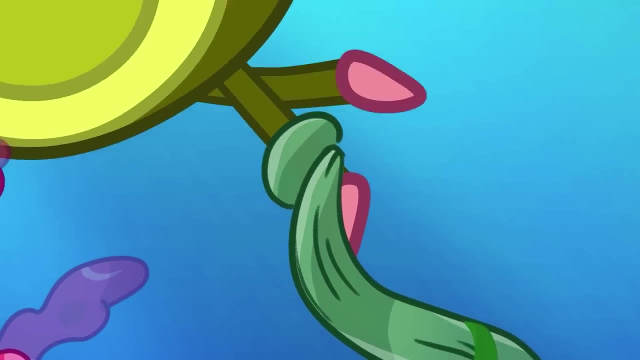 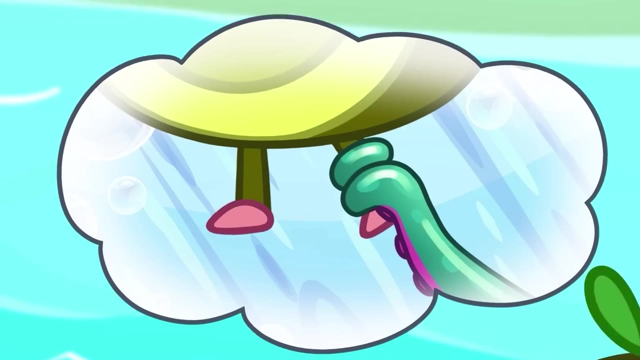 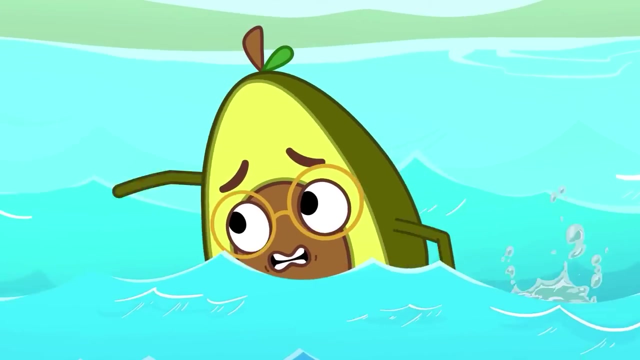 Penny loves swimming in the ocean. Oh no, Something grabbed her leg. Something grabbed her leg. She thinks it's a monster. She thinks it's a monster. Help me, Help me, Hurry, Daddy Penny needs your help. Hurry, Daddy Penny needs your help. 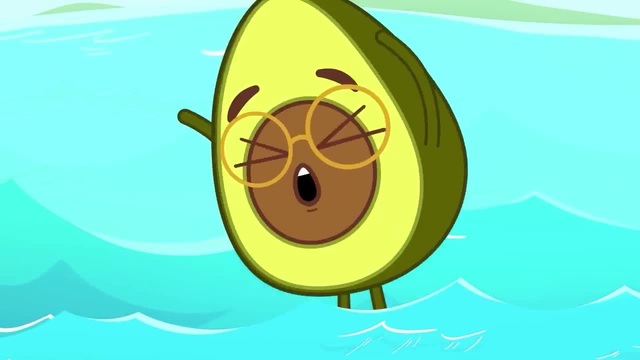 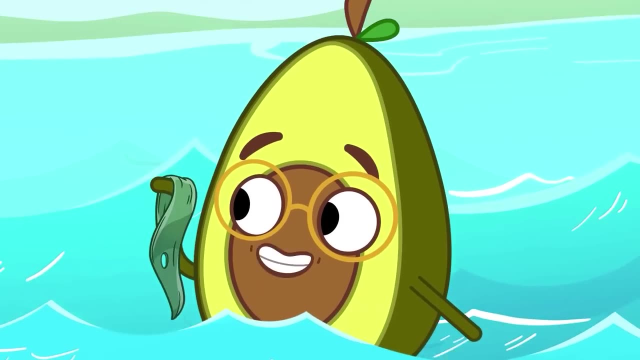 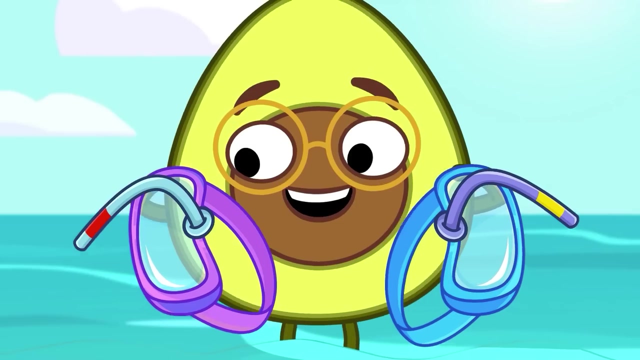 There is an underwater monster here. There is an underwater monster here. It's not a monster, These are sea plants. These are sea plants. Hehehe, Daddy has masks and snorkels. Let's take a look at the seaworld. 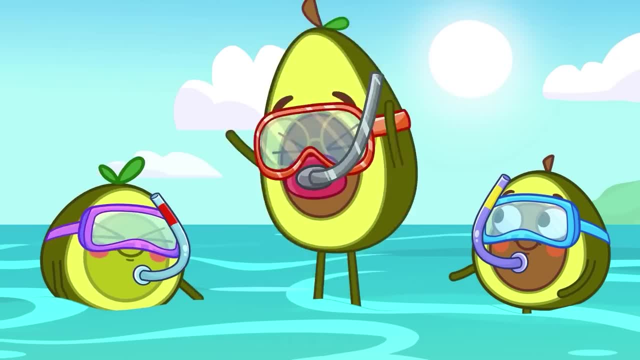 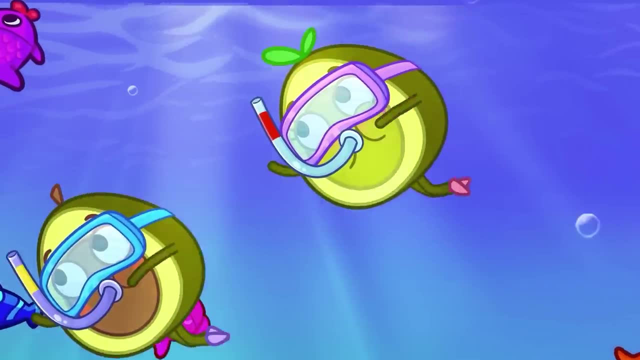 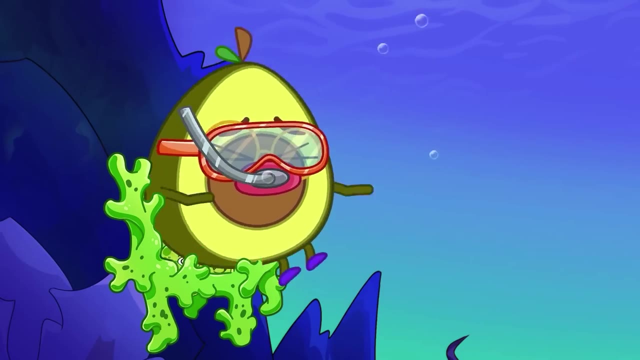 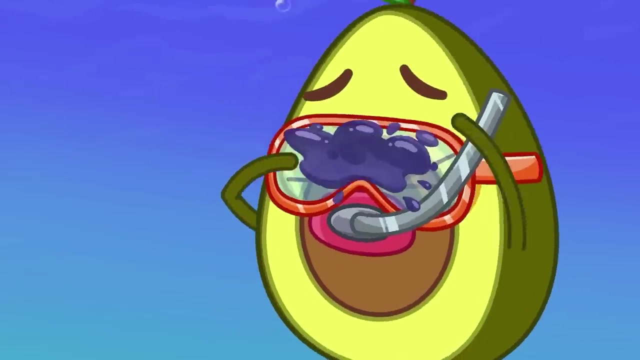 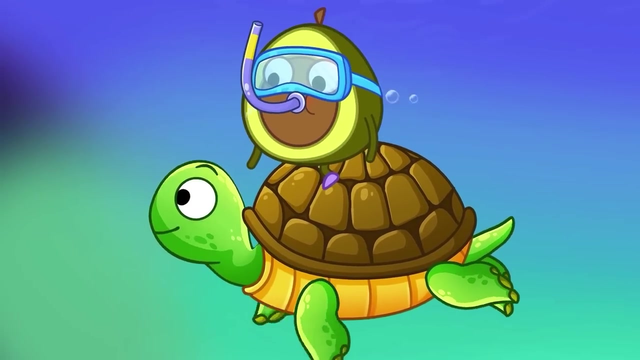 Let's take a look at the seaworld. Let's dive underwater. Let's dive underwater: colorful fish. That coral looks like a chair. Daddy sat on an octopus. It doesn't look very happy. Here comes the sea turtle, But you shouldn't ride on top. 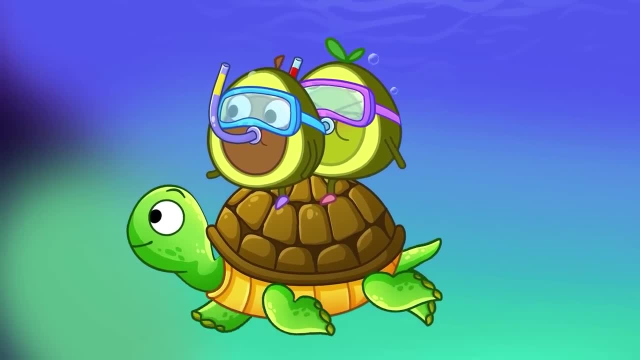 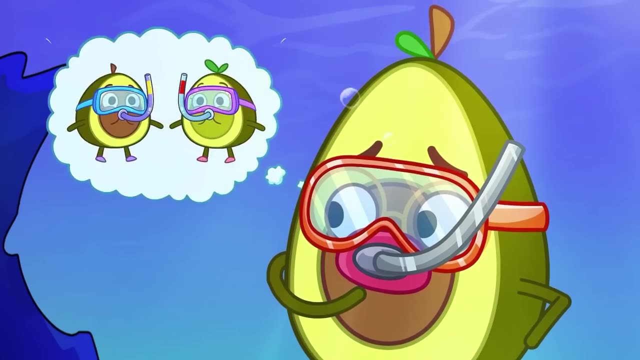 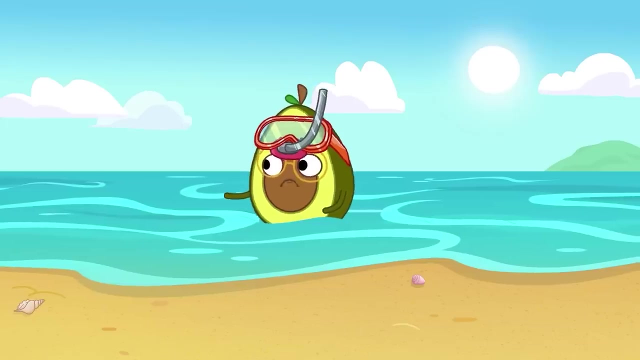 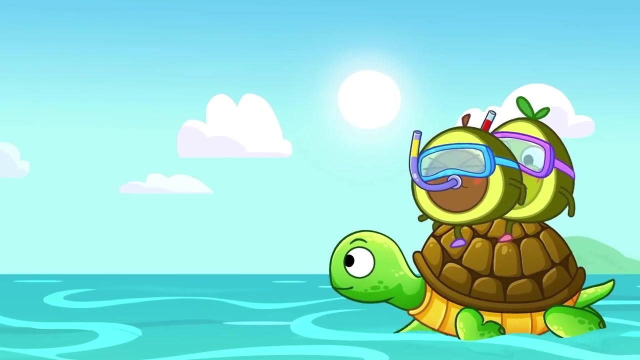 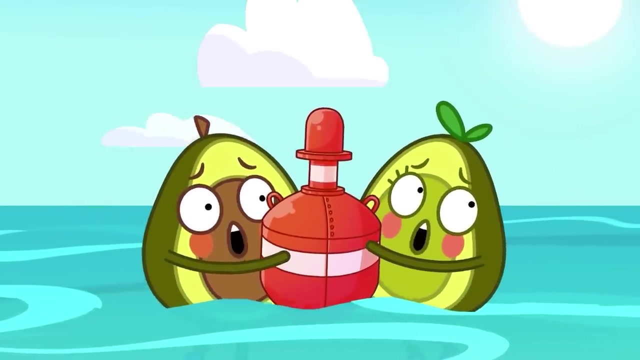 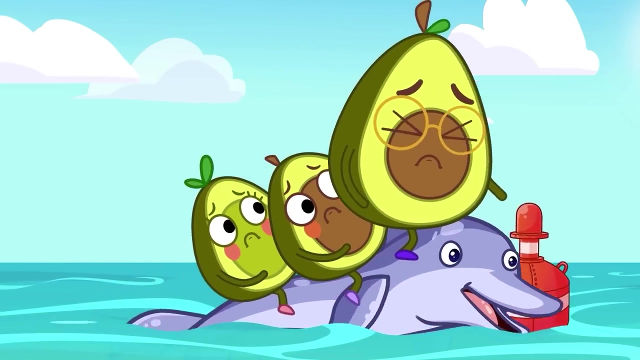 He'll take you far away from Daddy. Oh no, Now Daddy can't see Pit and Penny. Pit, Penny, Where are you? Here they are. They're lost and scared. Daddy, Help us. Here comes Daddy on a dolphin. He'll take everyone to the beach, Kids, it's. 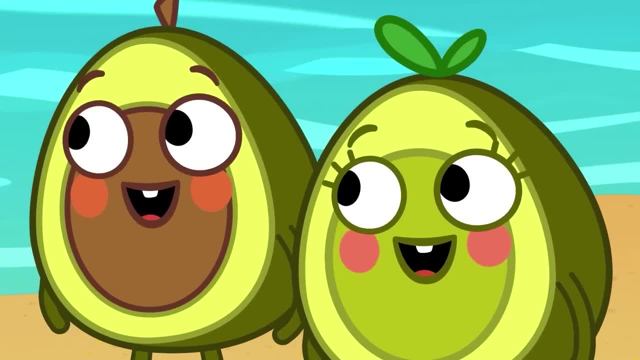 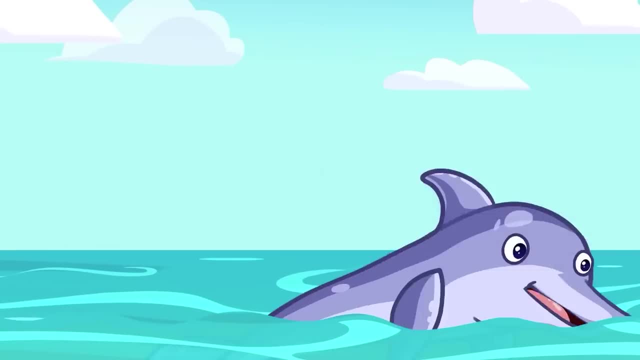 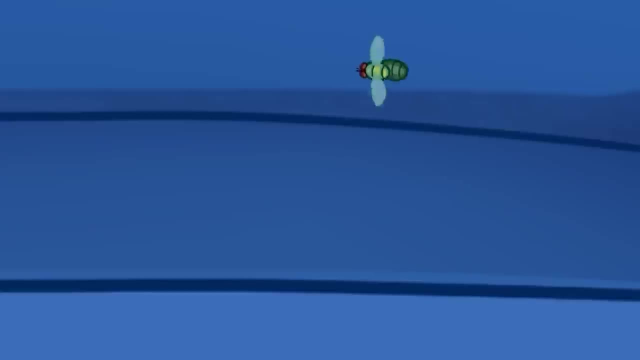 dangerous to swim far away from the shore. Always stay close to someone you know. Thanks, Mr Dolphin. Uh-oh, There's a fly in the house, But here comes Penny with a fly swatter. Penny, you turned the couch into gold. 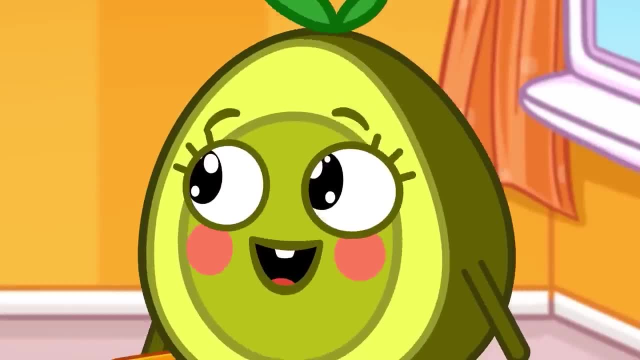 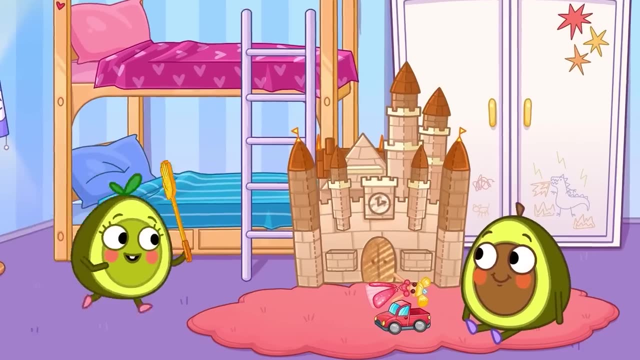 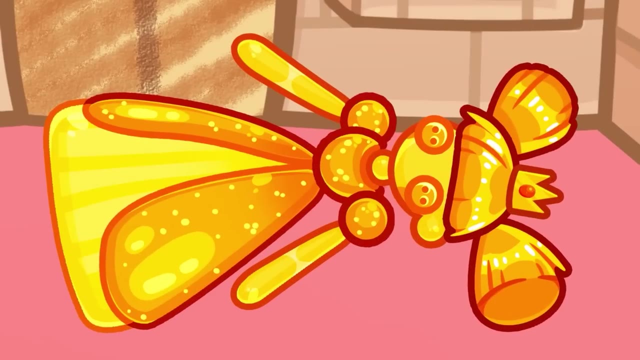 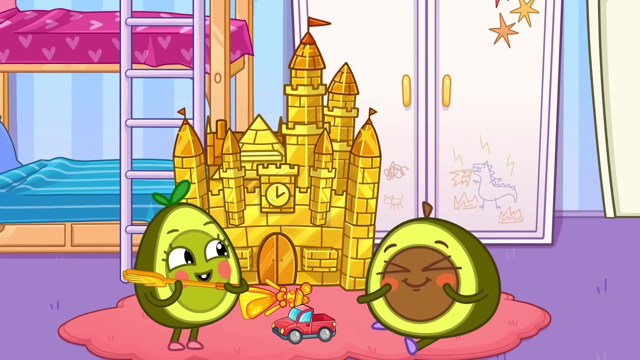 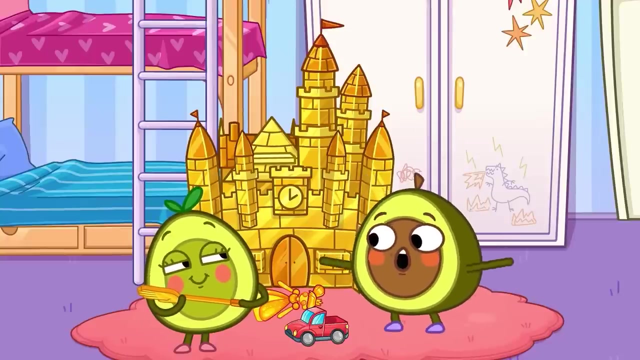 Now the TV and speakers are gold. Wow, The fly swatter is magic. Pit Penny has something to show you. Watch closely: Her doll turned gold And the castle turned gold. What do you think? Pit? Woo-hoo, Golden toys. Now do Pit's toy truck. 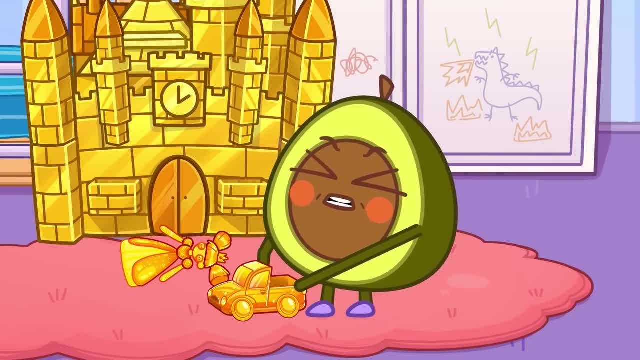 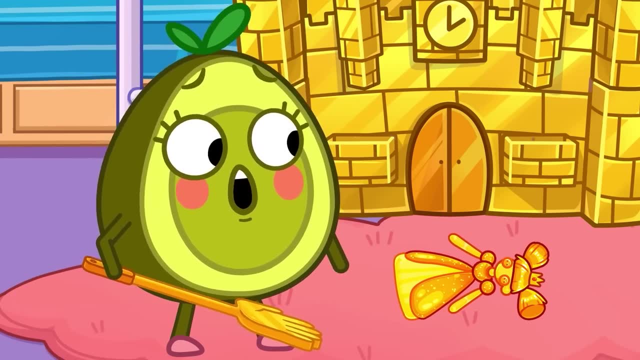 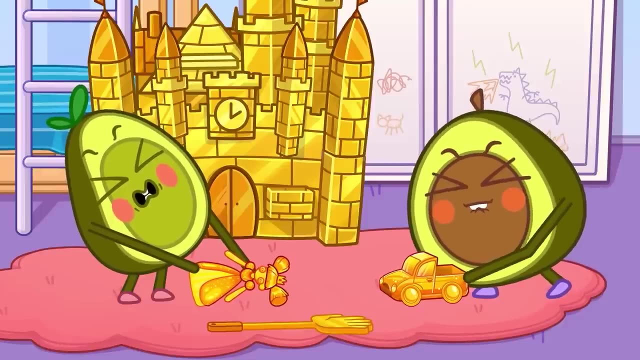 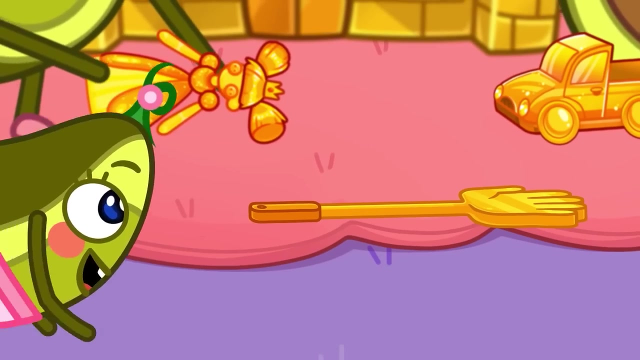 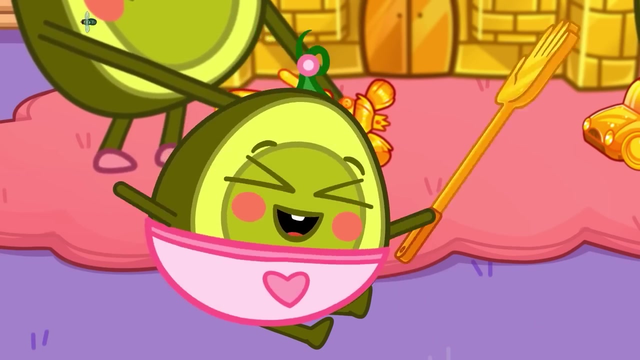 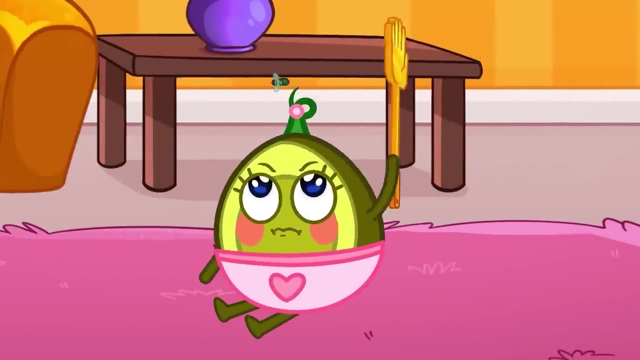 There's just one problem: Gold toys are very heavy. Try both hands. Penny, Hello Baby. And Baby wants the fly swatter. Careful Baby, The fly swatter is magic. Oh, Now there's a gold rod. 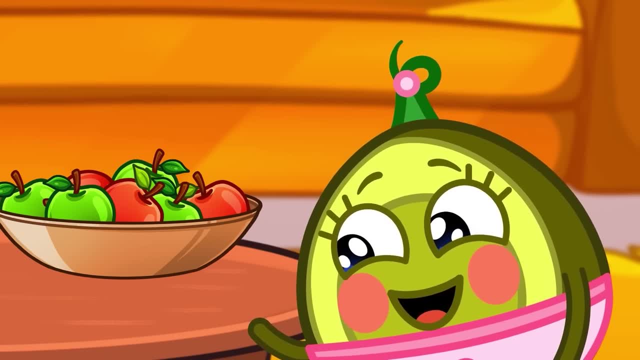 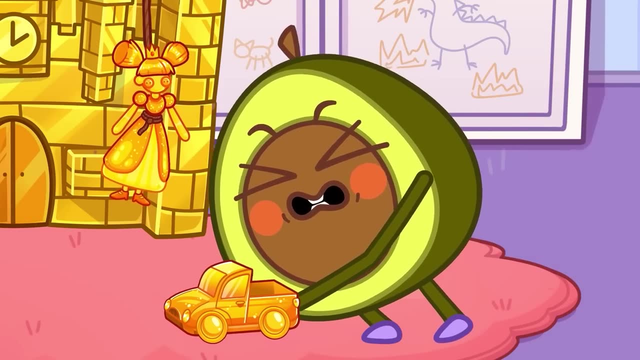 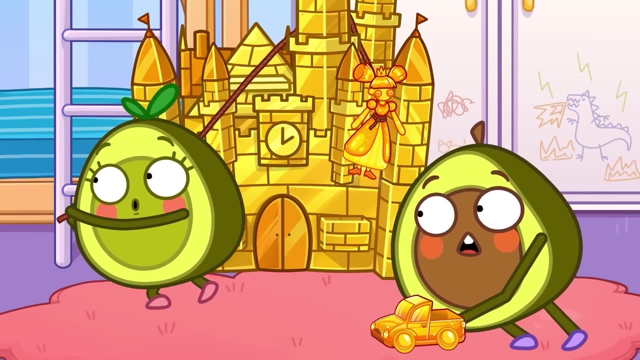 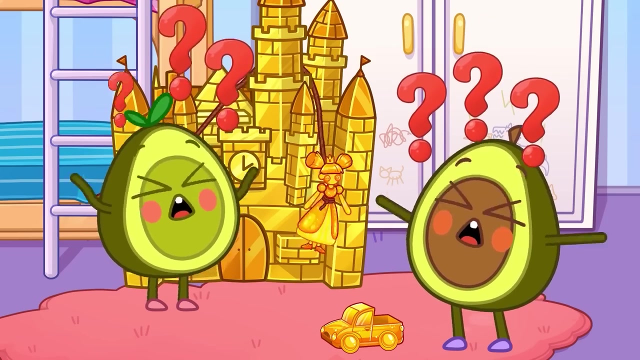 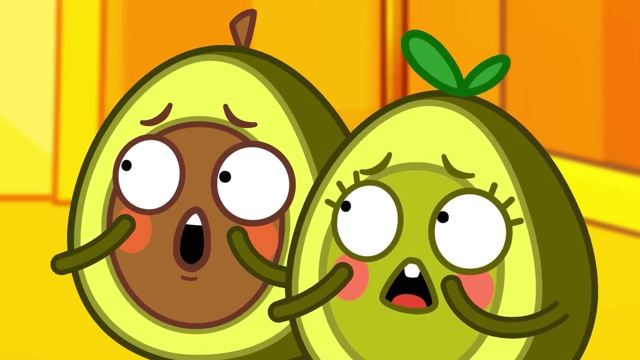 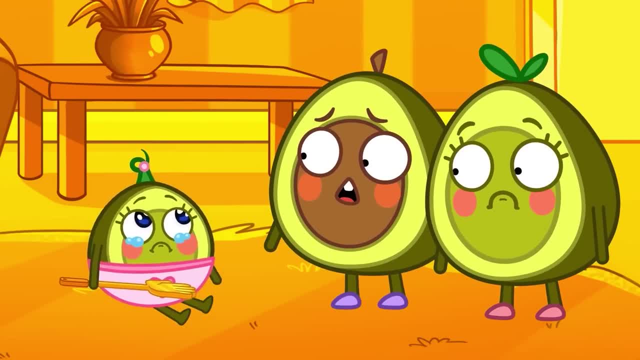 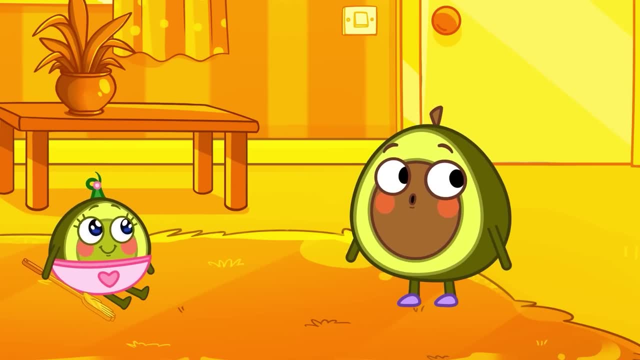 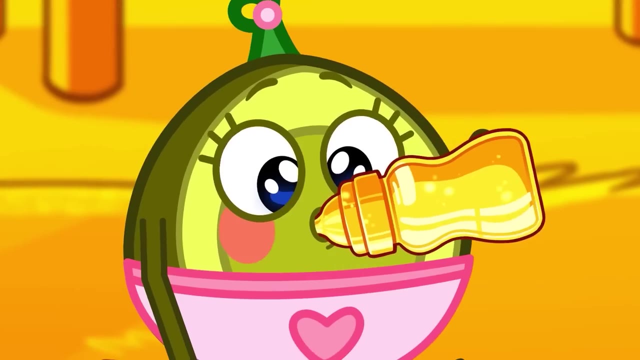 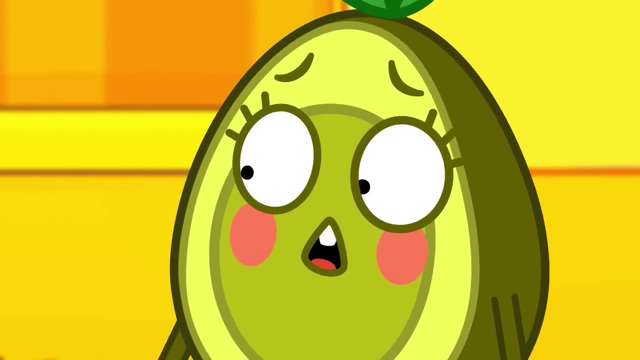 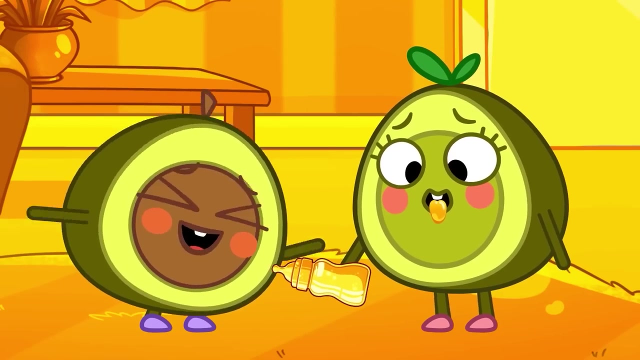 Gold, Gold, Gold, Gold, Gold, Gold, Gold. And Baby's hungry, Woohoo, She just wants her bottle. But the bottle is gold. There's even more, There's even more. Put some gold milk inside. 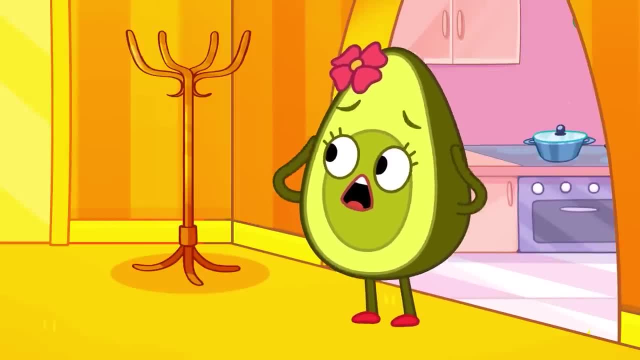 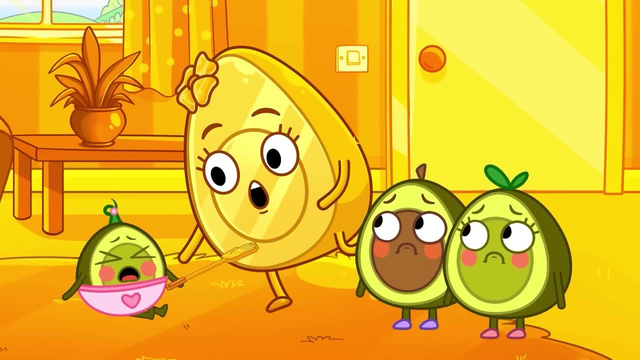 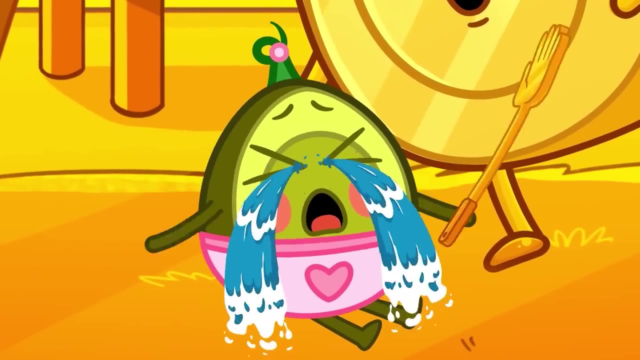 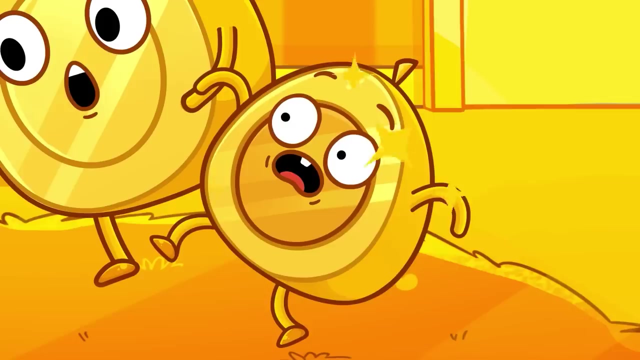 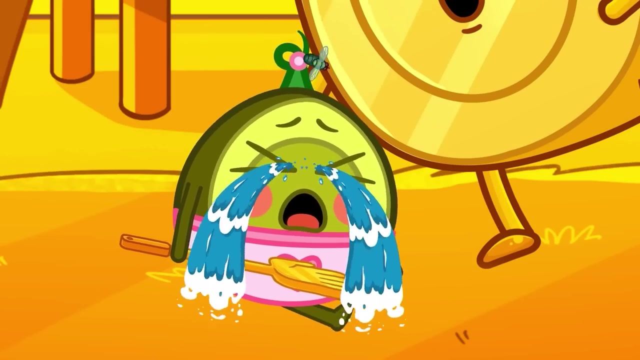 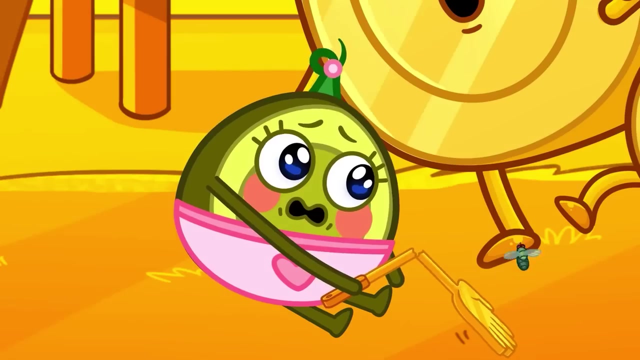 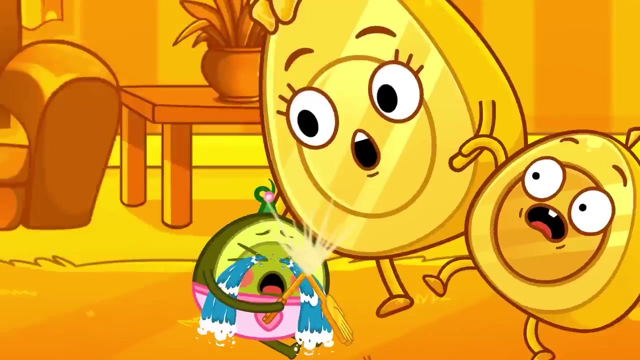 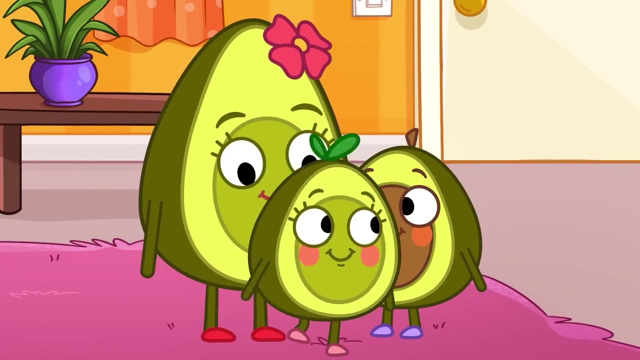 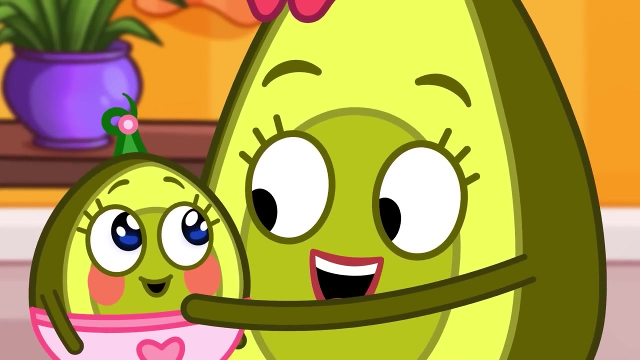 Maybe Mommy can help. Careful Mommy, Now Mommy's gold. Be careful Pits. It's been turned to gold too. Baby broke the flyswatter. Everything is back to normal, Oh, And you don't need this anymore. 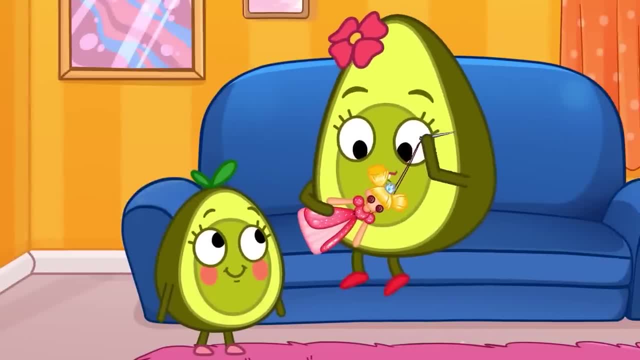 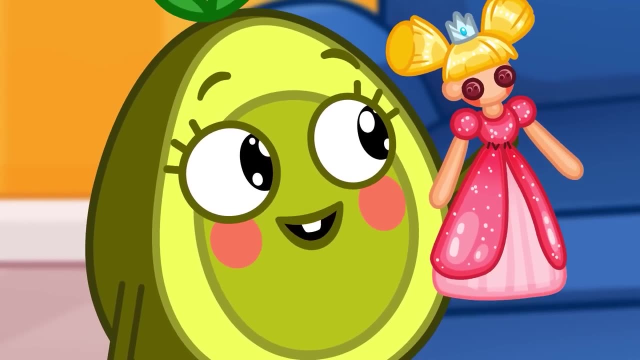 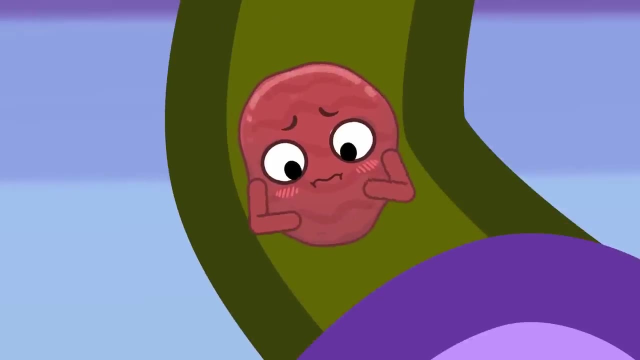 There, Penny's doll is back to normal. It's even better than gold. Hit has a scab on his leg. It itches so much, And Penny has a scab too. I can't stand it. Tear it off. 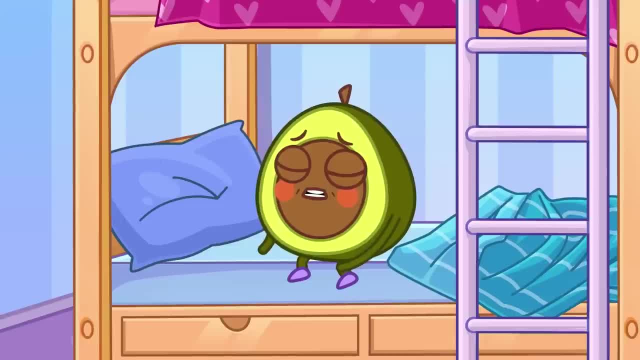 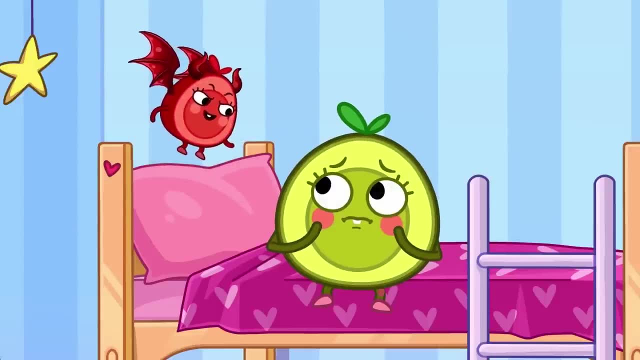 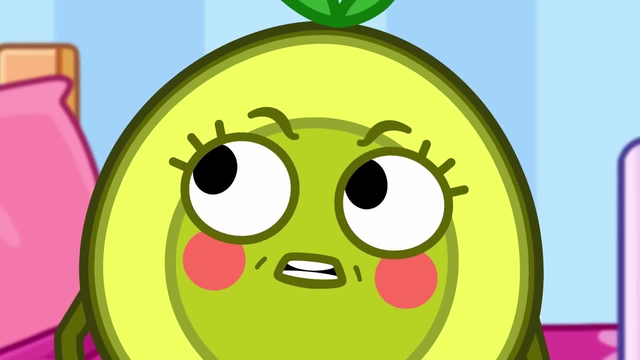 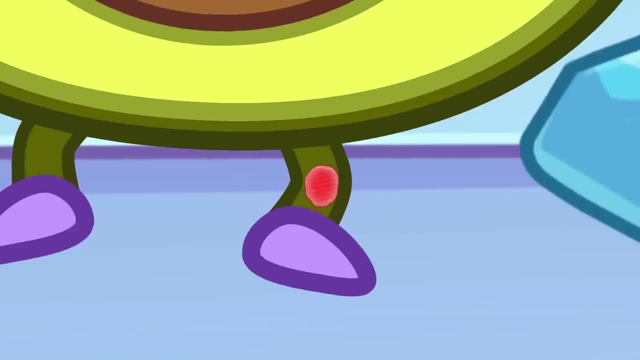 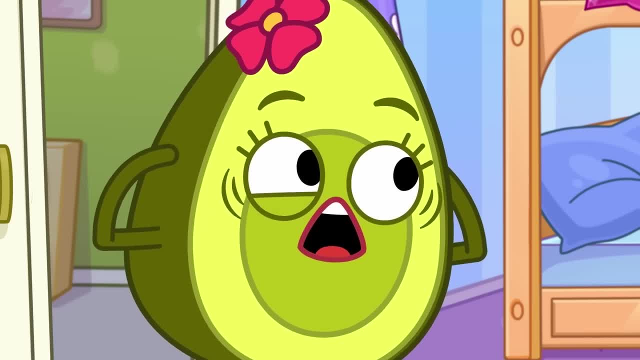 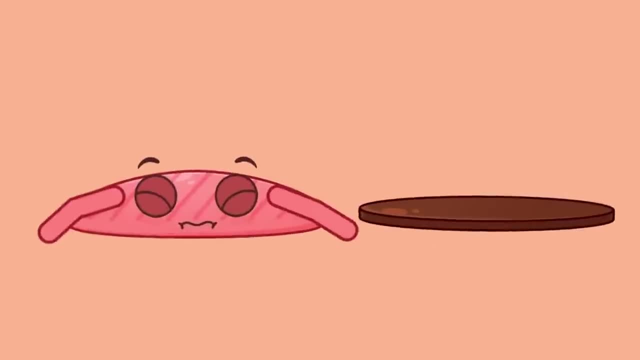 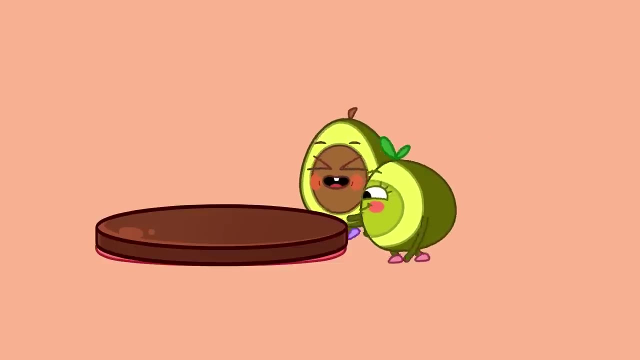 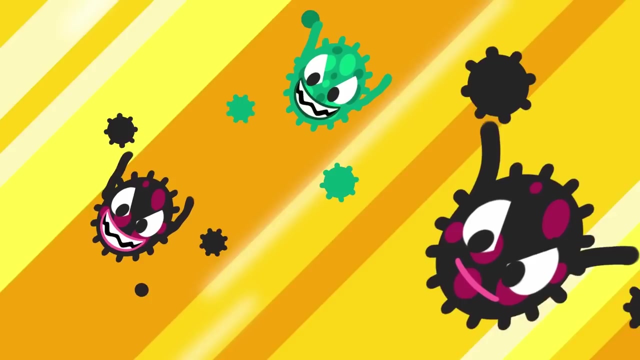 Oh no, Oh no, Mom, Mom, Mom, Oh, Di där, St Mentor ț See, This wound is protected by a scab, But if you remove it, bacteria can get inside it and make it worse. Wow, Brünnhild. Nope, You can't put a scab back on. We can't hold them back. What's that? It's blood platelets. They stick together and stop germs. They help make scabs. The wound is protected. So now your wound will heal much faster. 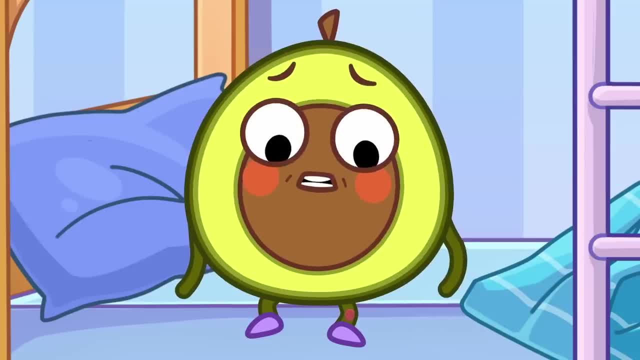 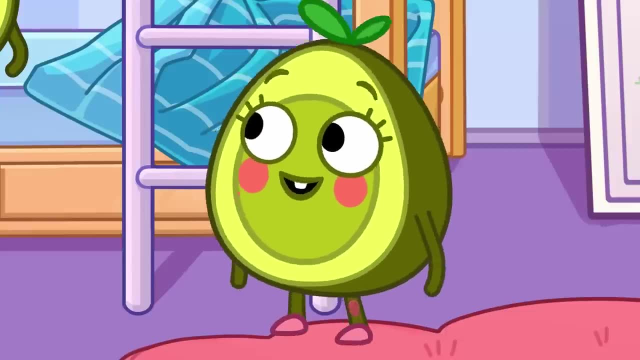 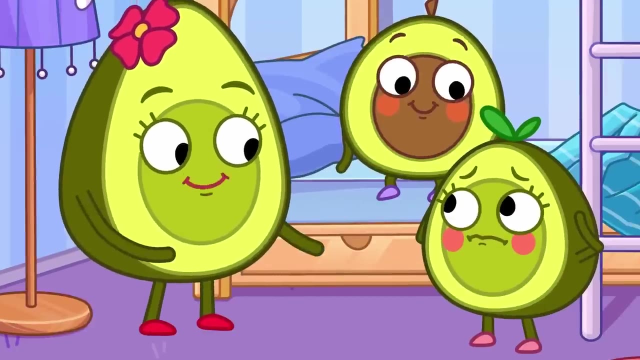 Thank you, mom. Leave it alone to heal, But it itches so much. This will help you Penny your scab. Oh no, My scab has fallen off, Don't worry. Now your knee is healthy. My wound healed faster than you thought. 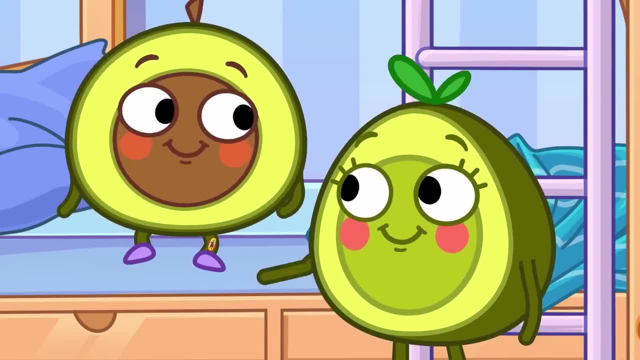 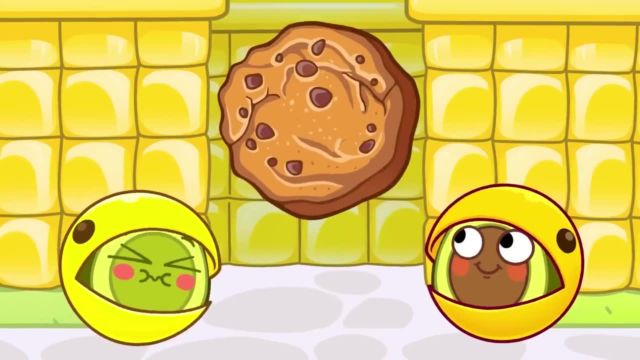 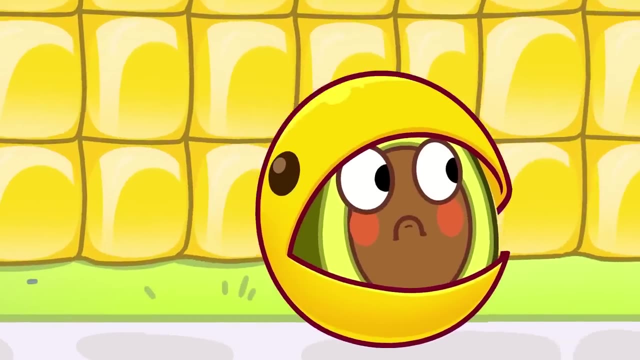 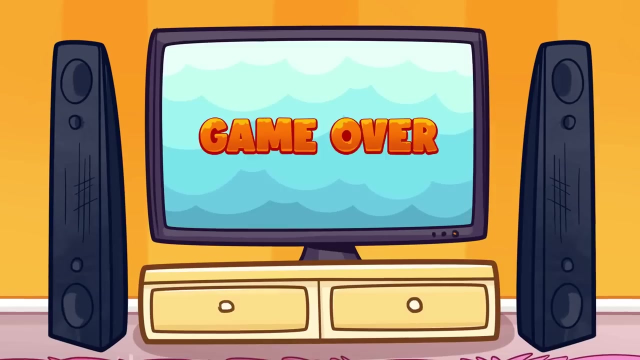 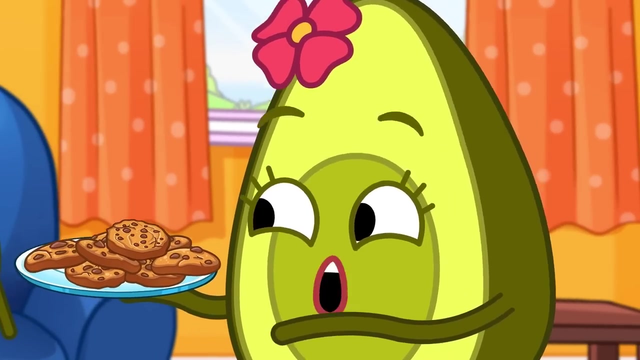 I will be patient until my knee heals. That's a great idea. Pit. Pit and Penny are playing a video game. Watch out for the evil cookie. Hurry Pit, Or it'll catch you. Oh no, Game over. Here are the cookies. 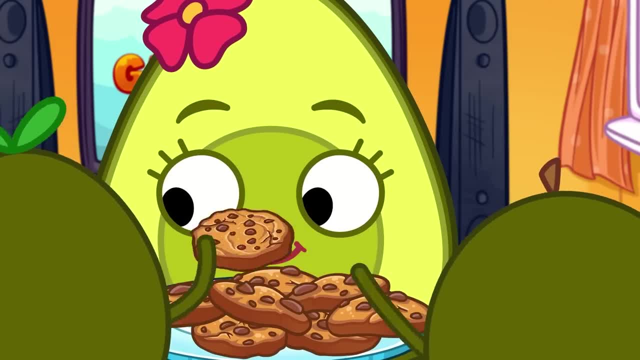 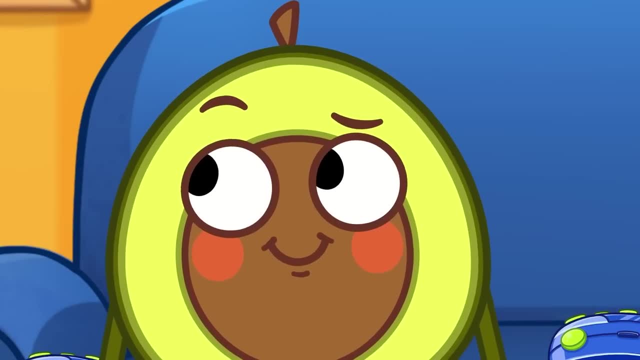 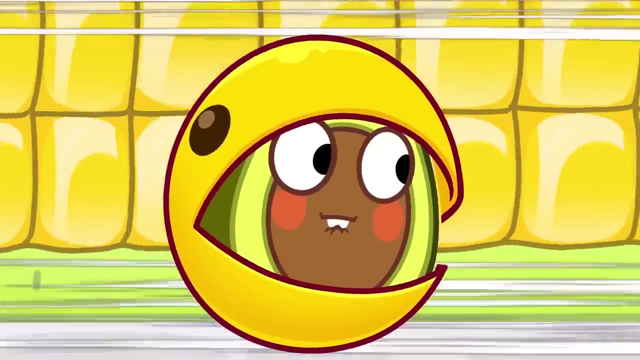 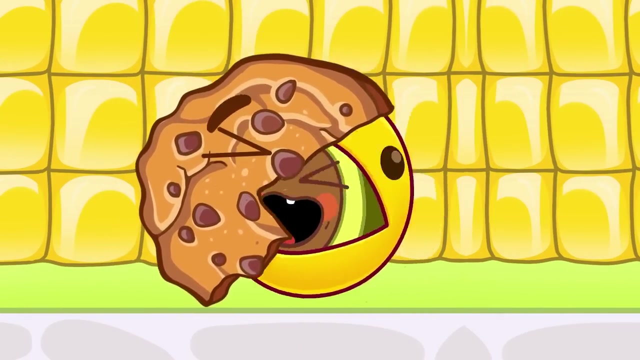 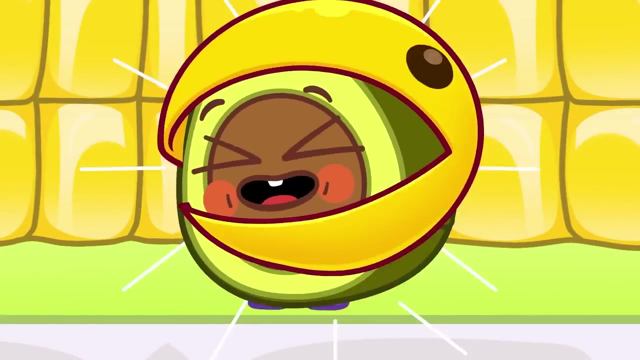 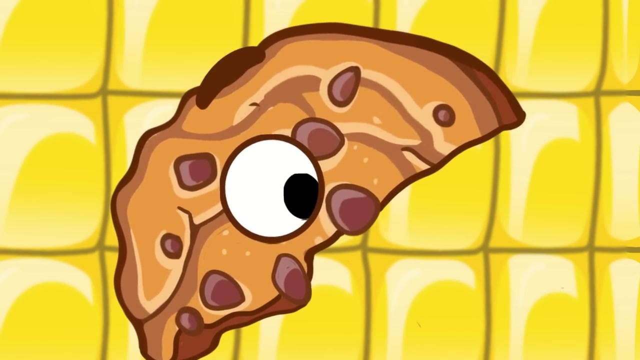 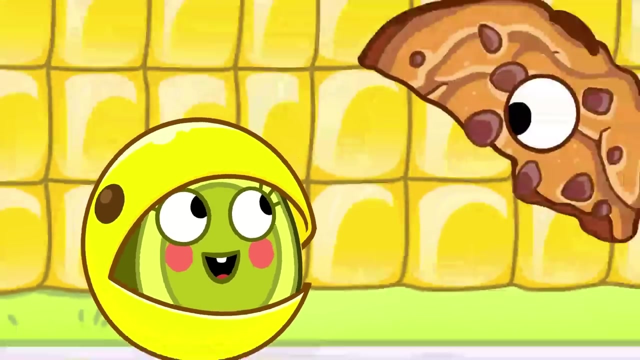 Yay, This gives Pit an idea. He'll just eat the cookie. Ooh Whoa, You got a cookie. It worked. You got a cookie. Woo Yaaay, Now Penny will eat the cookie. I'm gonna smile now, ha. 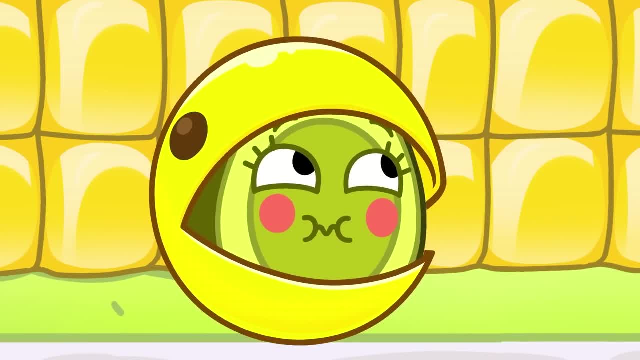 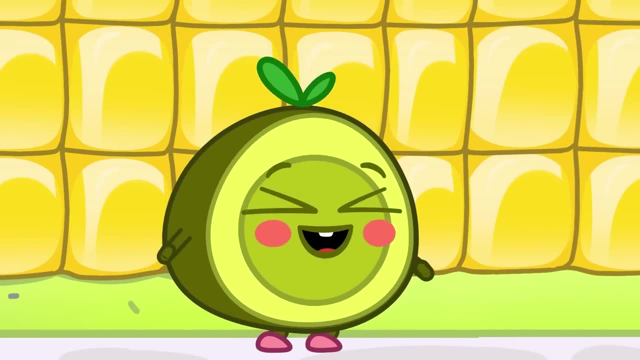 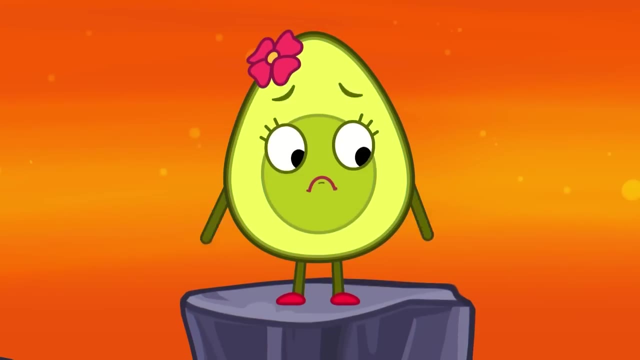 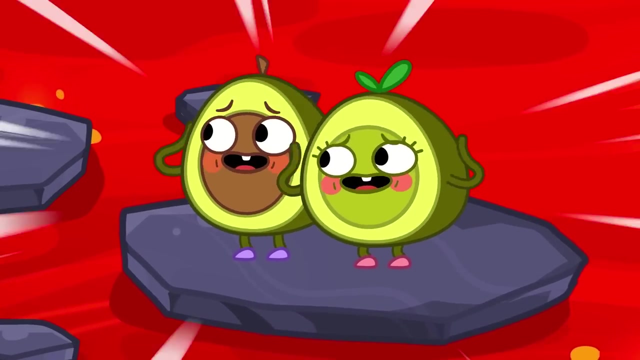 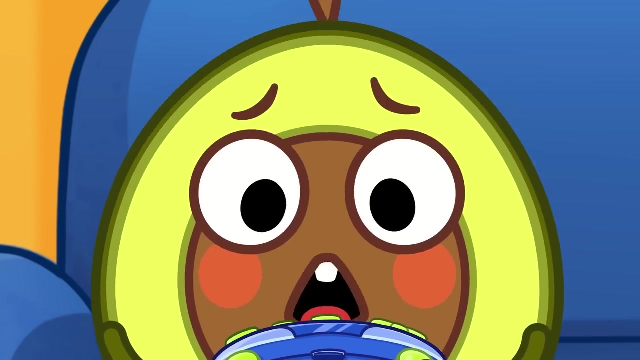 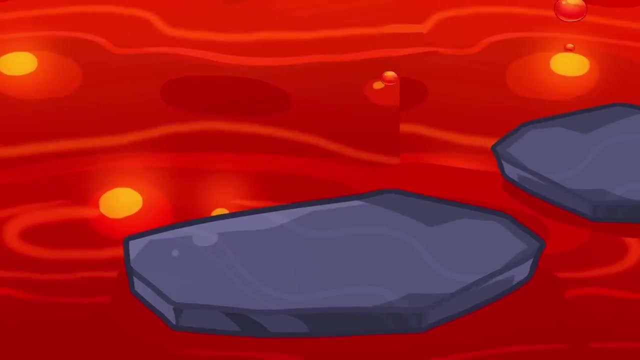 Take my cookie. Oh, You got a cookie. Yeah, Ah, You got a cookie. You got a cookie again. they made it to level two. oh, mommy's trapped and needs help. oh no, they've taken our mommy. oh, it's a burger monster. 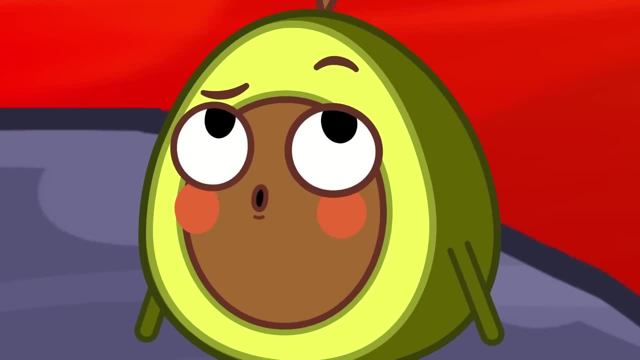 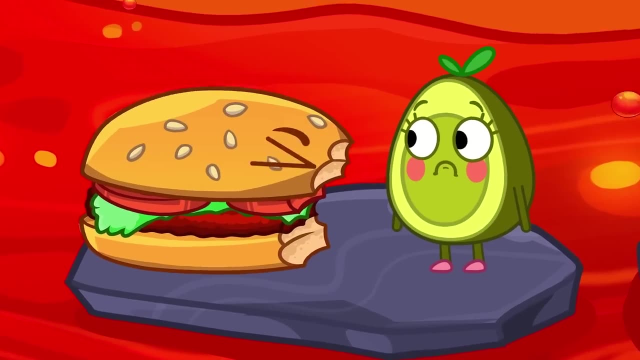 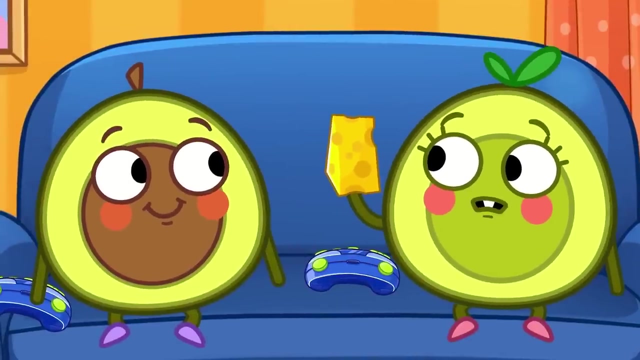 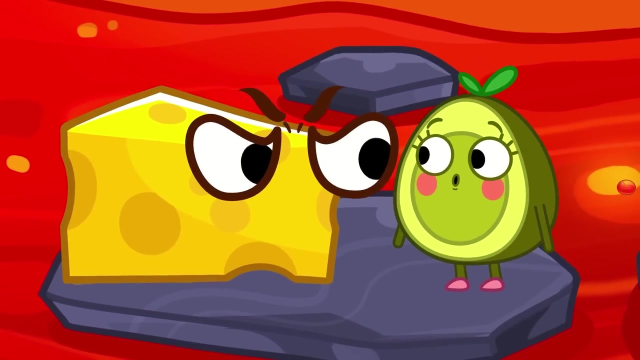 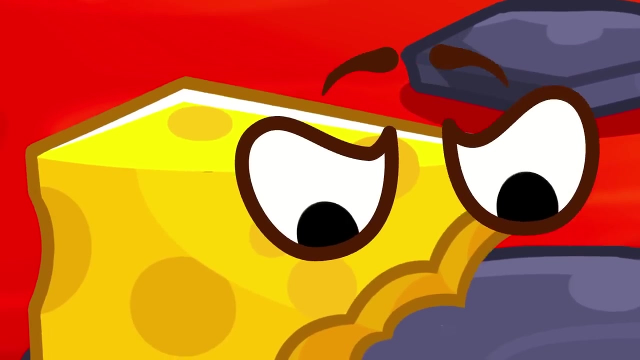 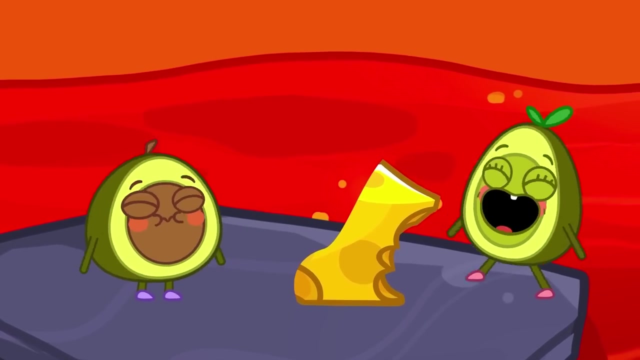 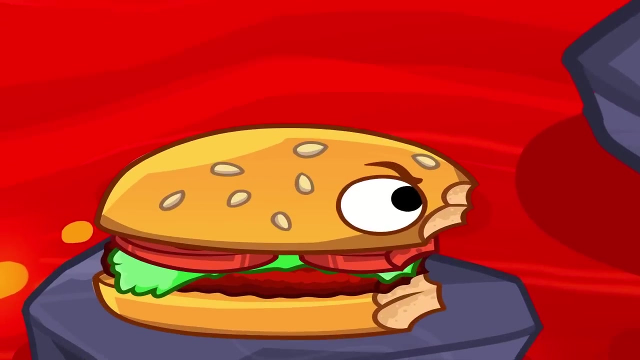 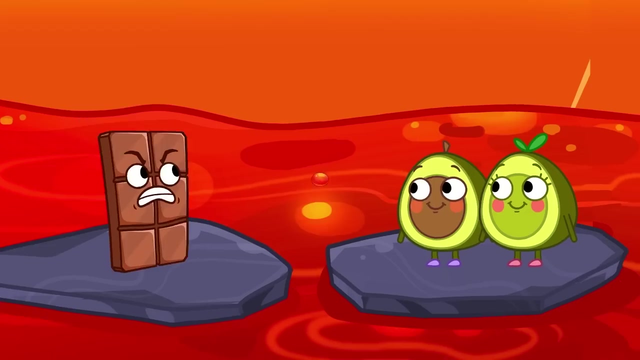 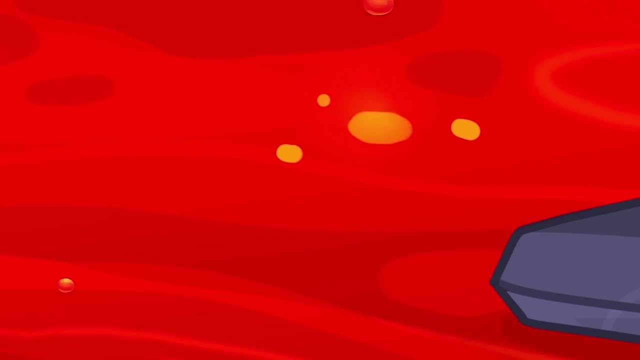 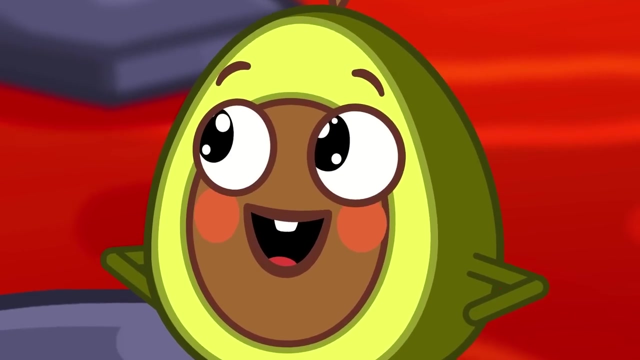 oh, no pitt is losing energy. what are you going to do, penny? healthy foods, give us strength. Cover up on healthy snacks like cheese. Now you have more energy. Now you have more energy. Yay, You saved Mommy. Victory, It's the final round. 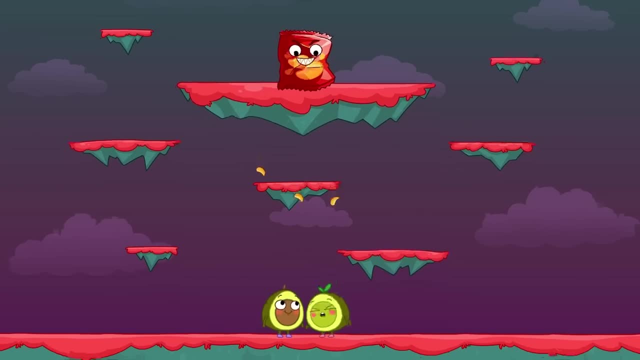 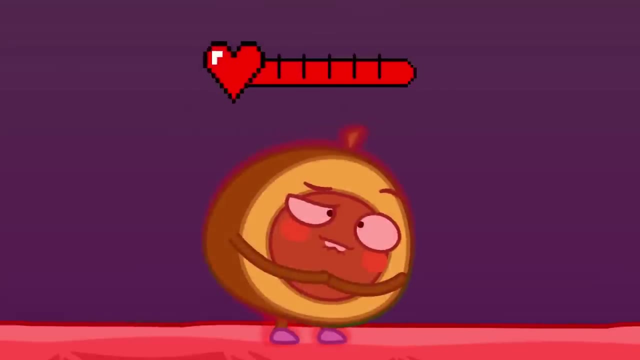 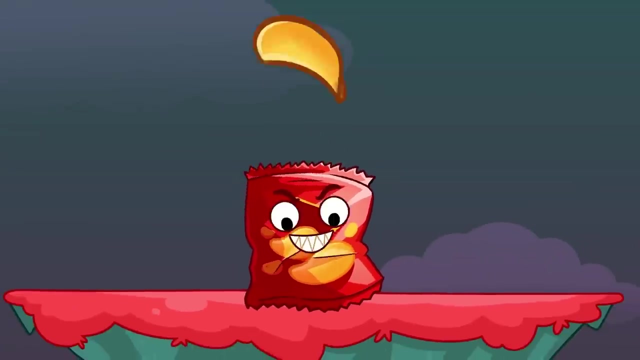 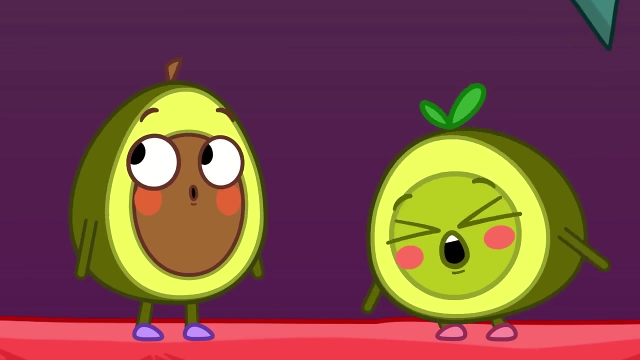 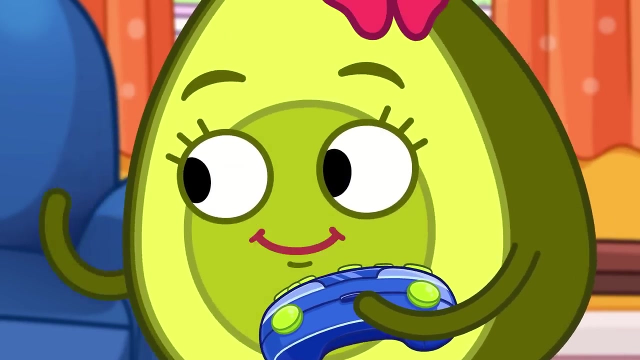 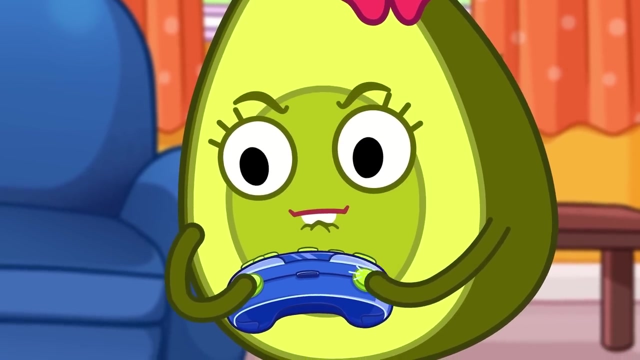 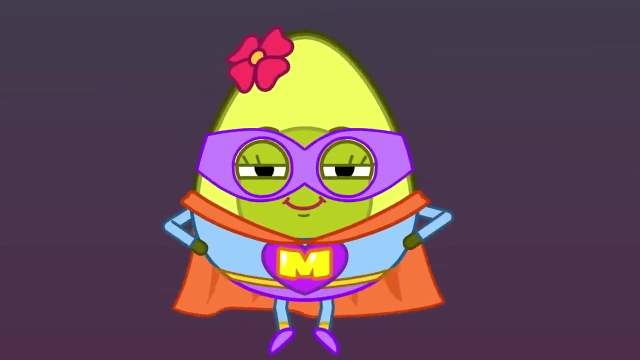 The kids must defeat the evil bag of chips. The kids must defeat the evil bag of chips. Pit lost some energy. Watch out, Super Mommy, to the rescue. I will help you. I will help you. Okay, Pit and Penny. 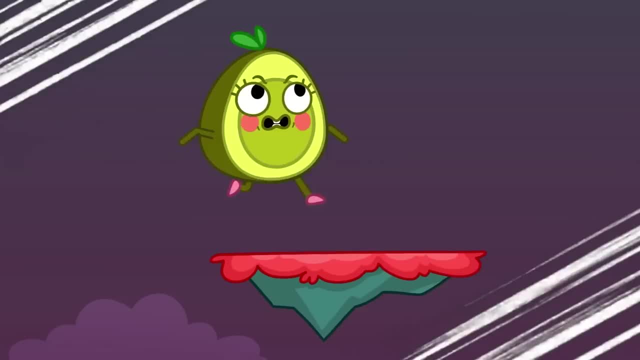 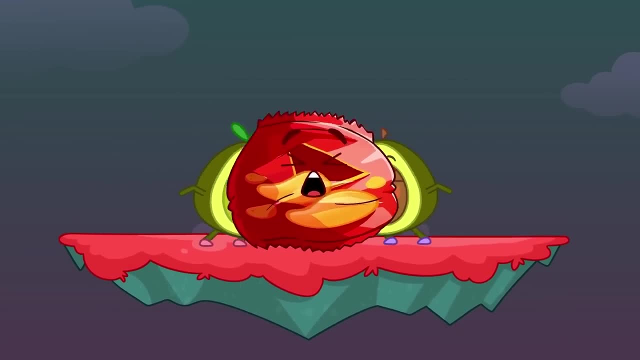 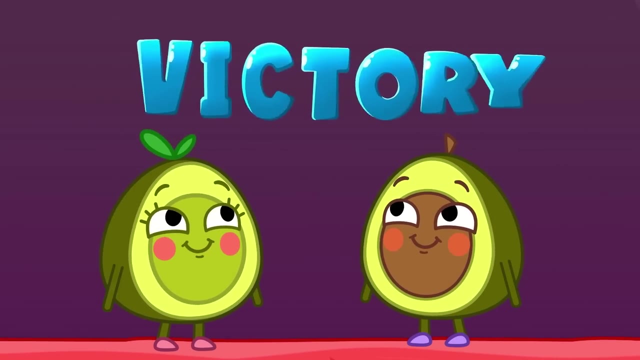 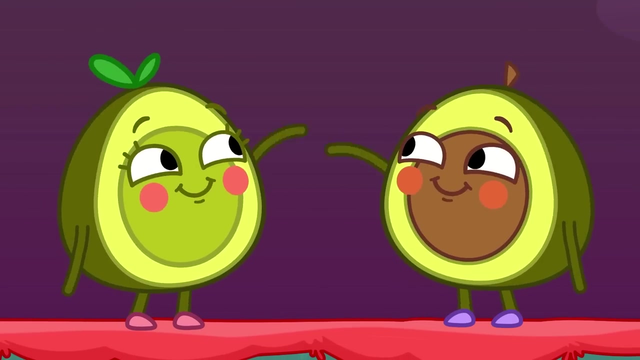 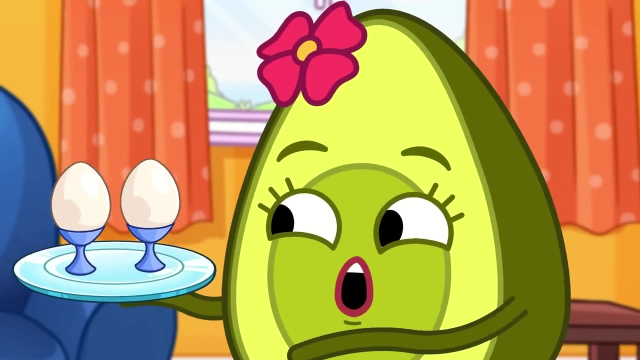 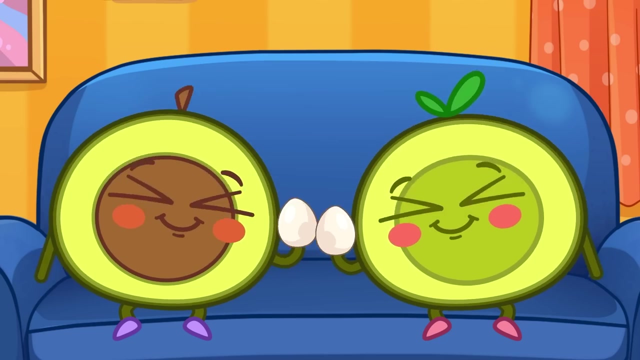 It's your turn. You won. You won the game. Mommy has a special treat for you. Mommy has a special treat for you. Healthy food makes you stronger. Healthy foods like eggs, Yum. Have fun kids. Have fun kids. 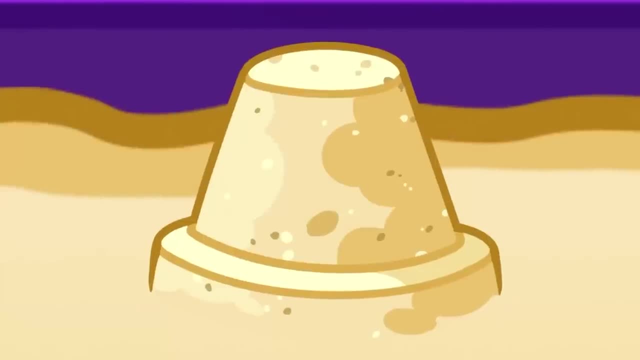 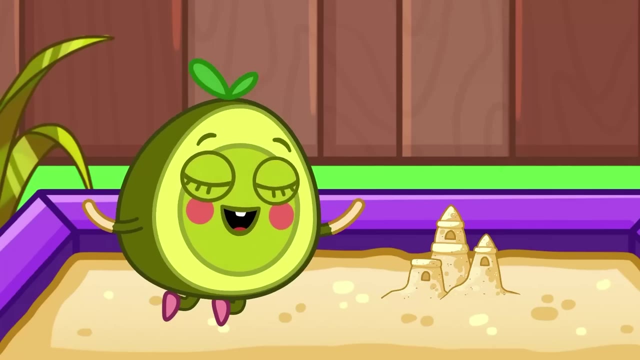 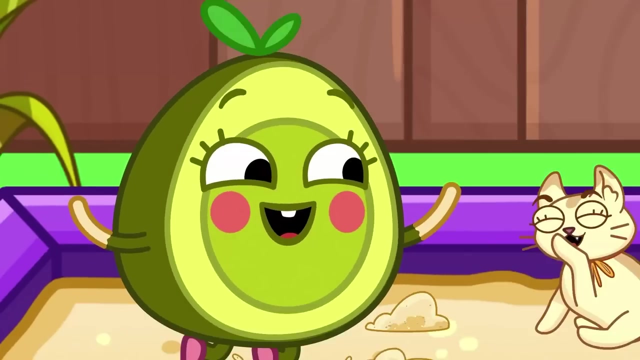 Penny is making a sand castle. Have fun, kids. It needs some work. Good job, Penny. Good job, Penny. Oops, The kitty ruined the castle. Oops, The kitty ruined the castle. But he's so cute. But he's so cute. 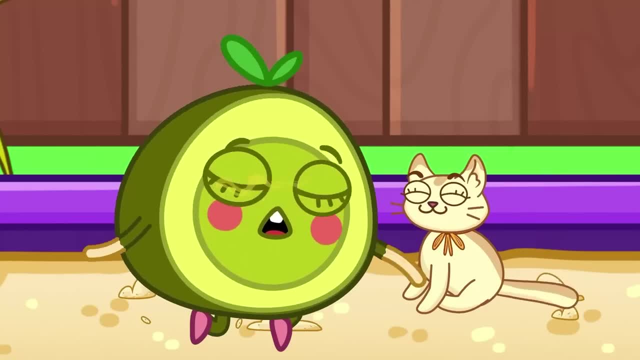 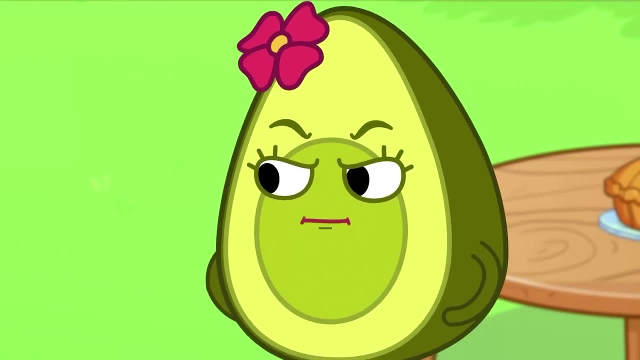 Mommy made a yummy pie. Mommy made a yummy pie. Mommy made a yummy pie. Have you washed your hands? Have you washed your hands? You should never eat food with dirty hands. You should never eat food with dirty hands. 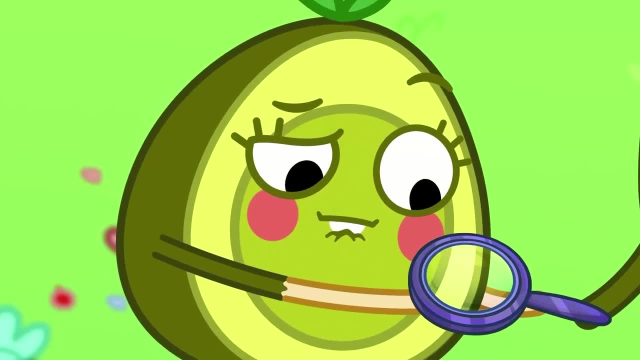 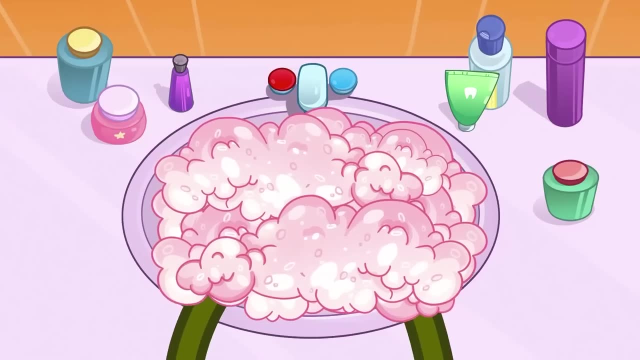 See all the germs. See all the germs. Penny, we can sing and wash together. Penny, we can sing and wash together. Soap, soap bubble bubble water splash splash. Soap. soap bubble bubble water splash splash. 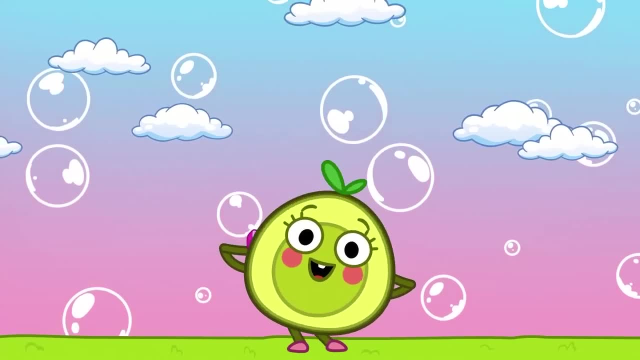 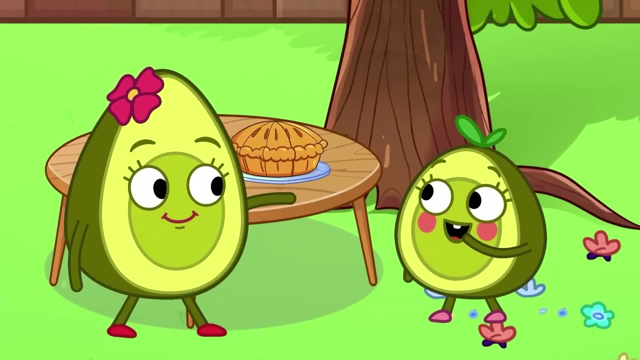 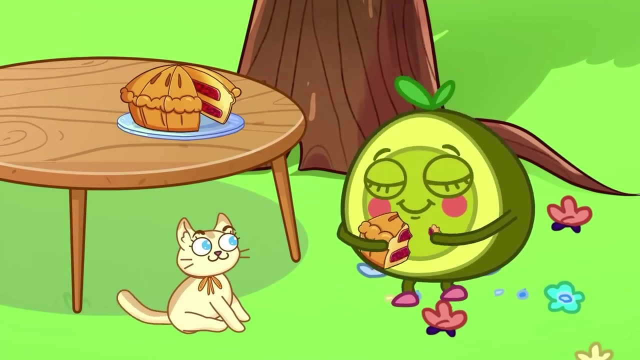 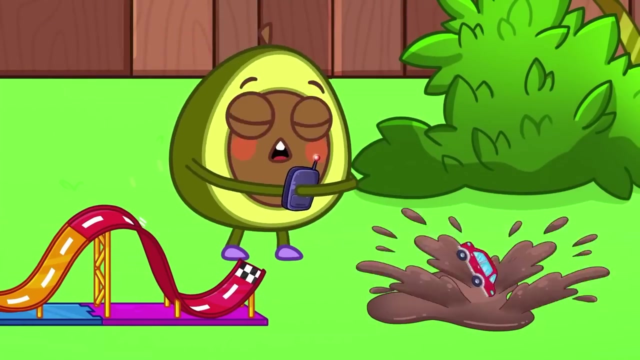 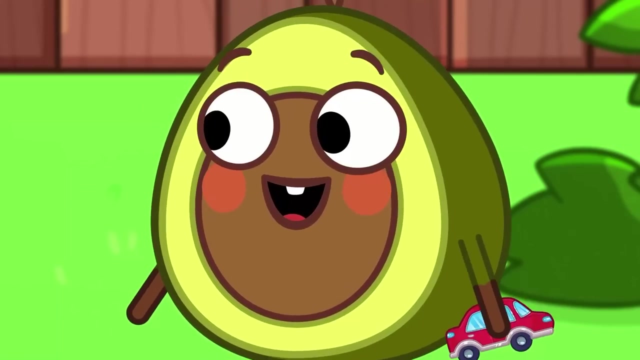 Welcome to the clean hand steam. See, Mommy, All clean. Now Penny can have some pie, And here's some pie for Kitty. Yum Pit is playing with his car, But now it's all muddy Pit wants some pie. 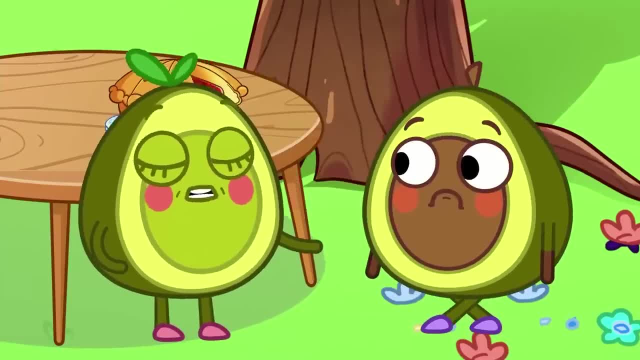 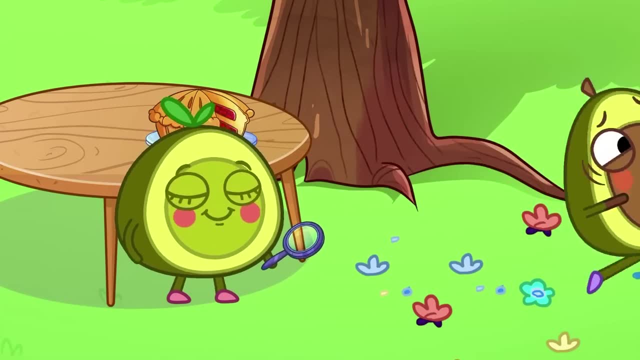 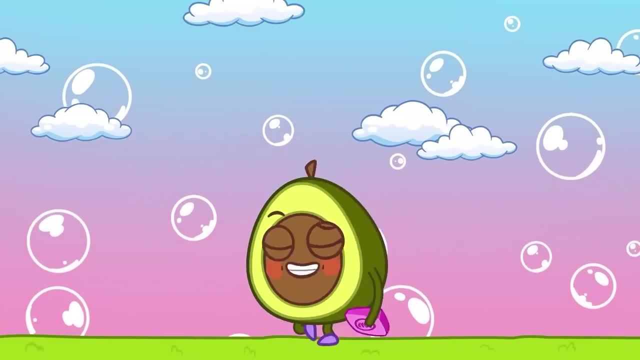 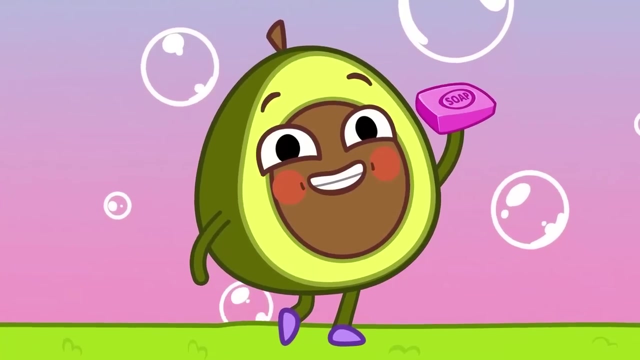 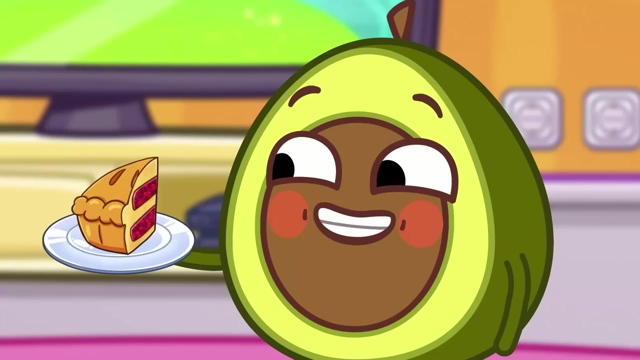 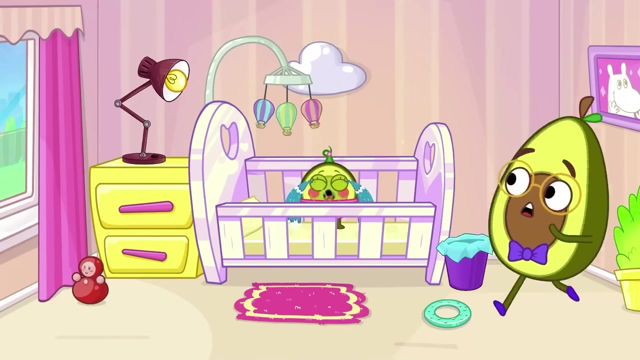 Wait, Pit, You need to wash your hands. They're covered in germs. see, Let's sing Now. Pit's hands are clean And here's some pie. Baby is crying. Daddy is here to help. Baby needs a diaper change. 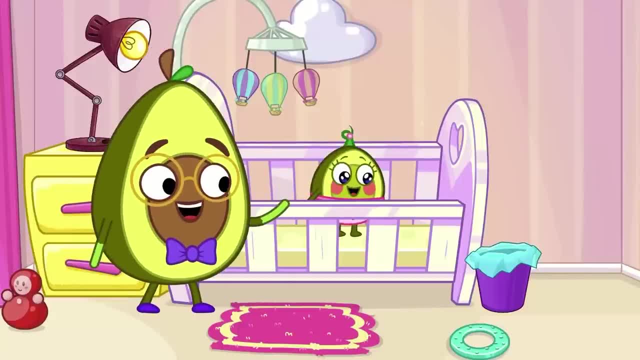 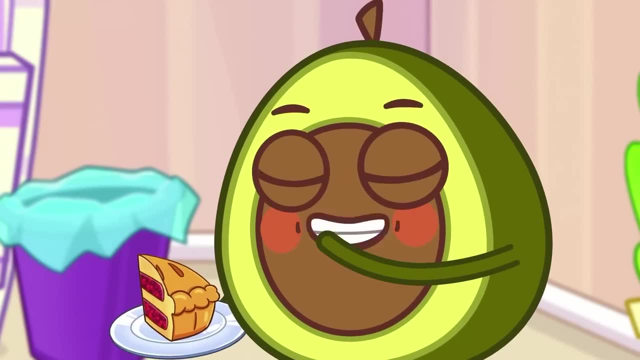 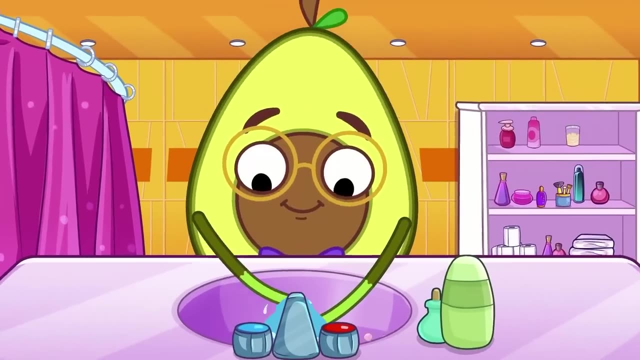 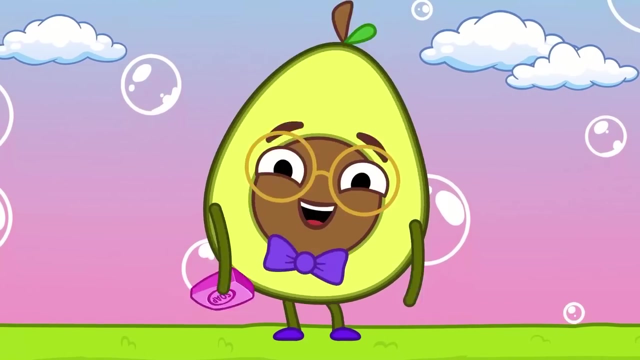 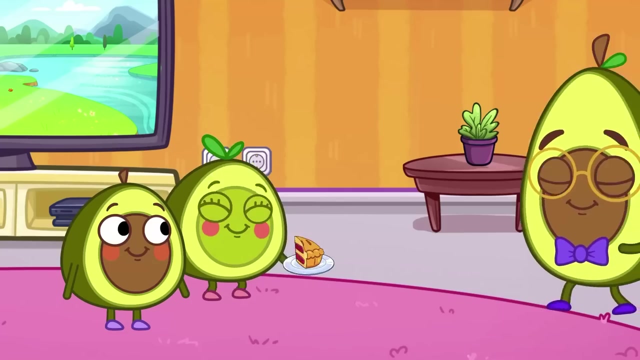 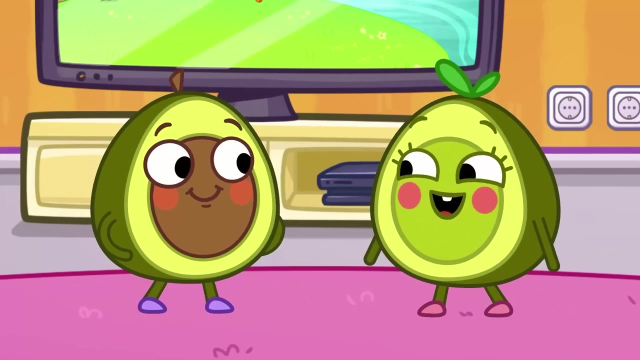 That's better. Now Daddy wants some pie. Wash your hands, Wash your hands. Even Daddies have to wash their hands. Let's all sing. Daddy's hands are all clean. He can have his pie now. Well done, Pit. 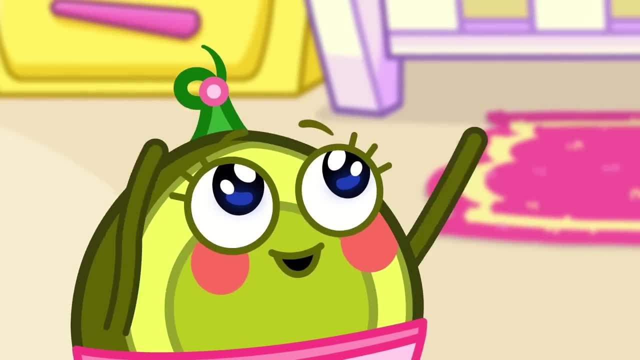 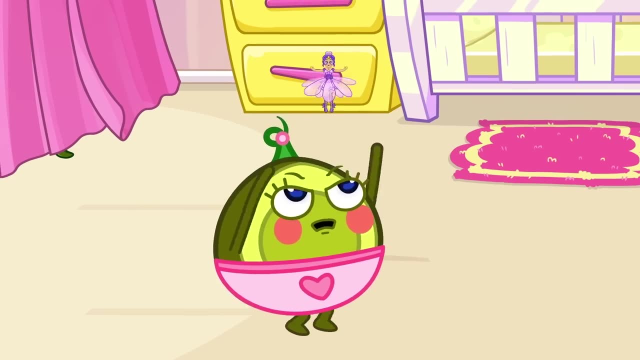 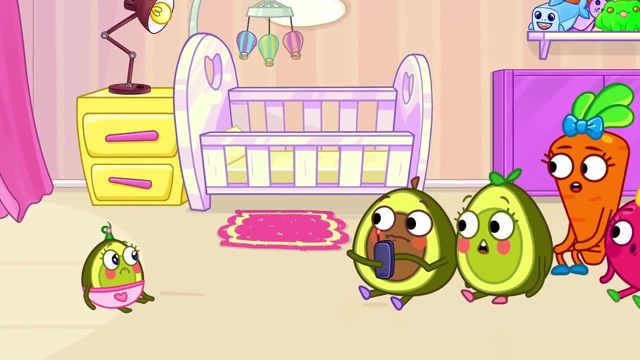 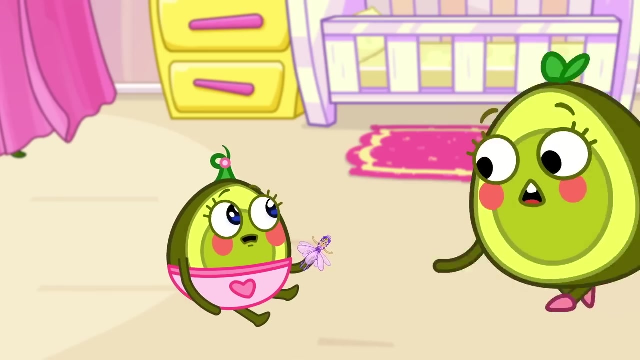 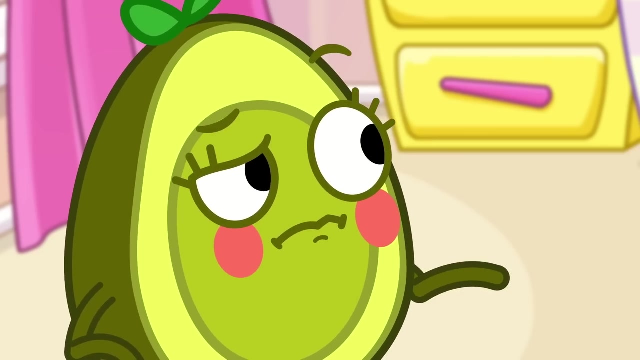 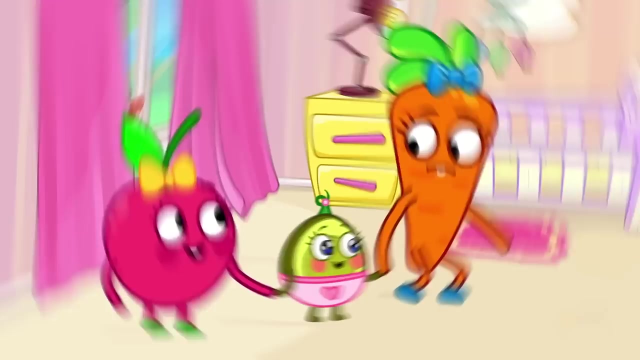 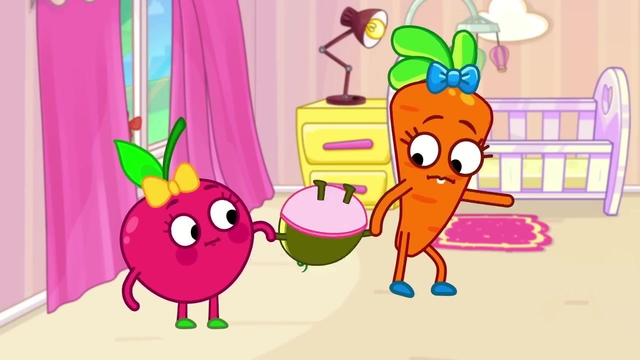 Well done, Penny. Baby wants the fairy doll. The kids thought it would make her walk. Baby's happy now Happy. now I know what to do. Holding Baby's hands might work. Nope, that didn't work at all. Let's try it my way. 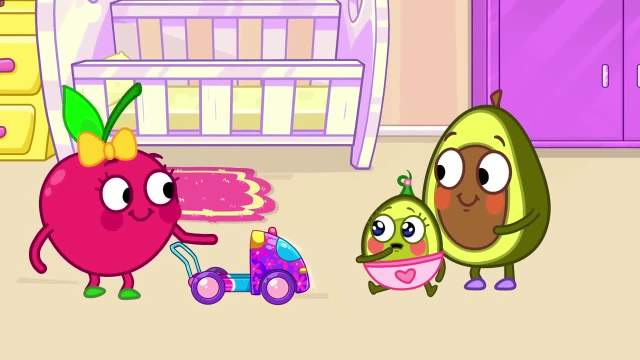 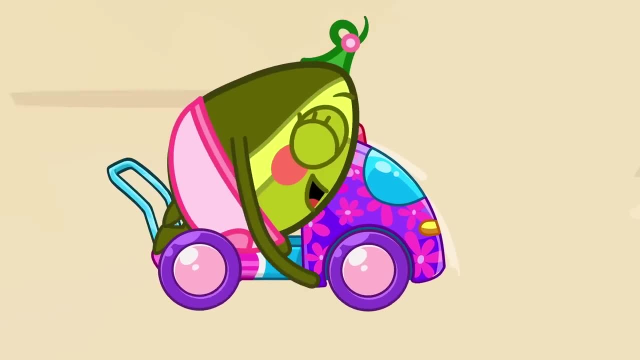 The toy might help Baby. The toy might help Baby walk. We're going to get a little bit of fun. Let's do it, Mommy, Let's go Baby. Do we have a ball? No, Choose one Oh. 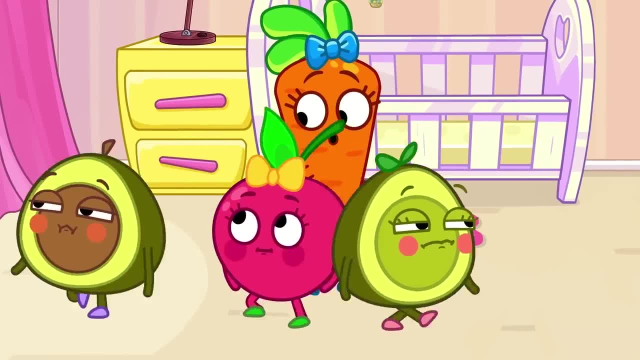 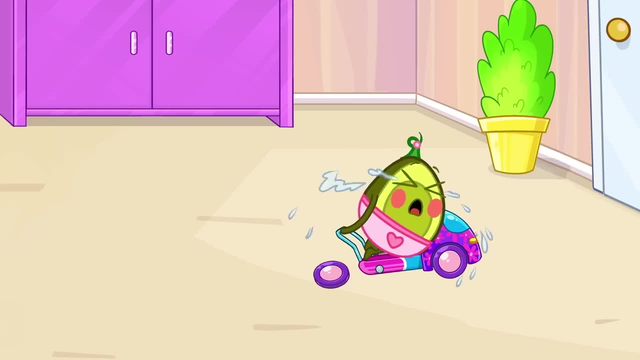 Let's just go Baby Yeah, All right, let's go E-e-e-e-e-e-e-e. Up Up, Up, Yeah, Up, Up, Up, Up Yeah, You're going to be under a lot of pressure. 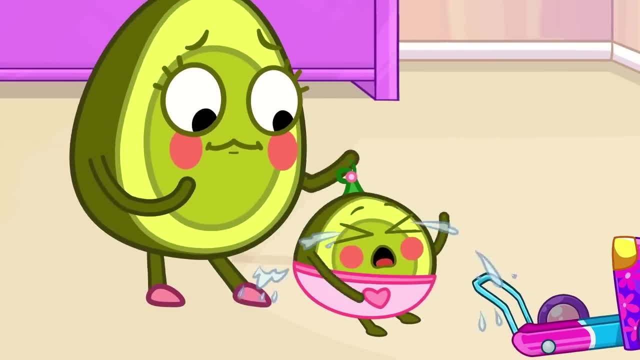 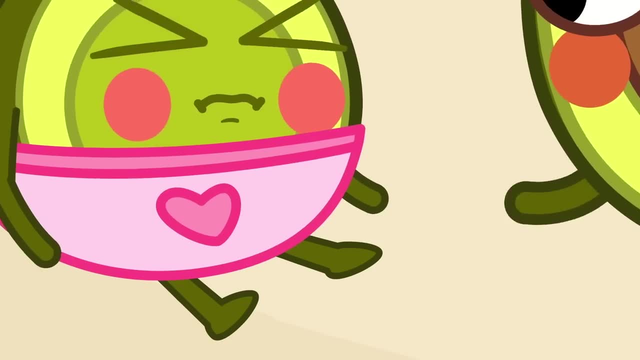 Oh good, You're going to be under a lot of pressure. Yeah, Yay, Oh yeah, Yay, Yeah, Yay, Yay, Yay, Yay, Yay, Yay, Yay. What are you thinking Pit? 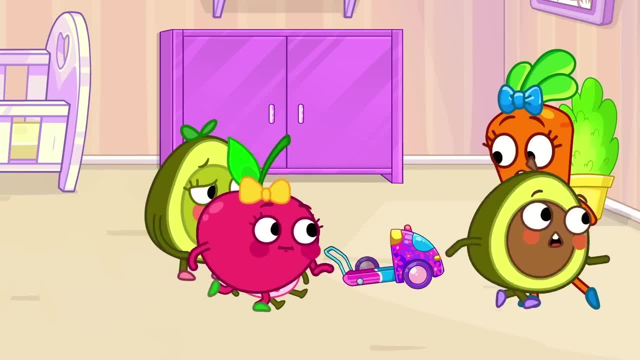 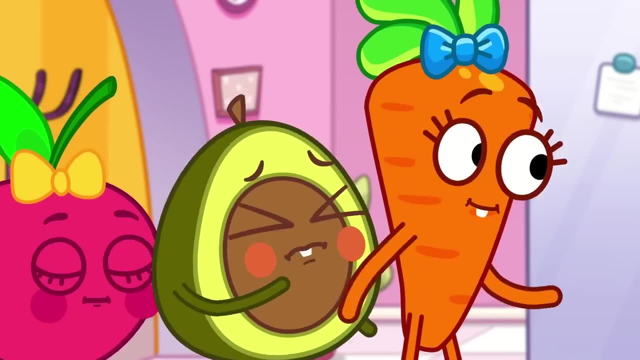 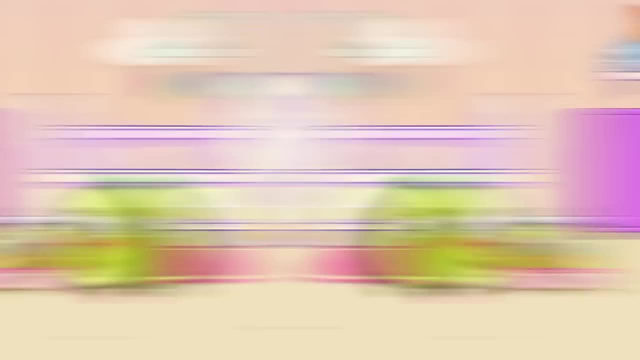 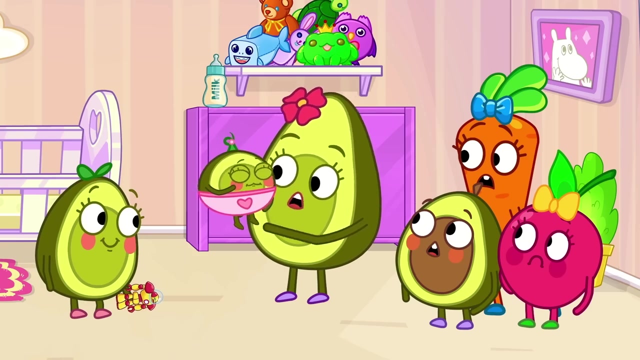 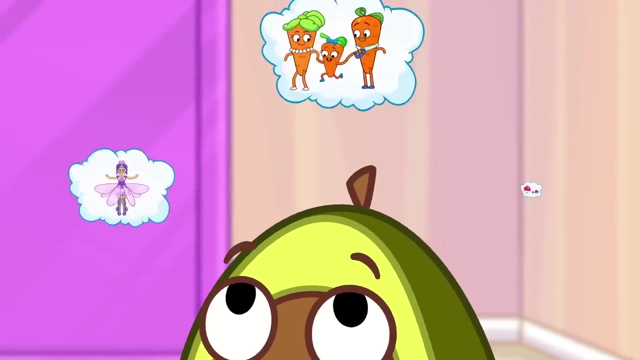 It's clear She's broken. Mommy, the kids are worried. Baby is broken. Baby is broken. Where does it hurt? We've tried everything but she can't walk. Mom, let's call a doctor to fix it. 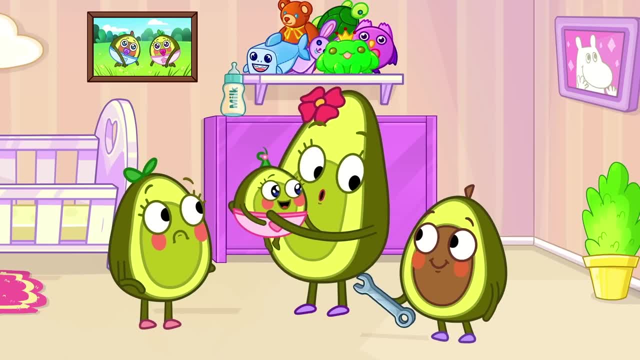 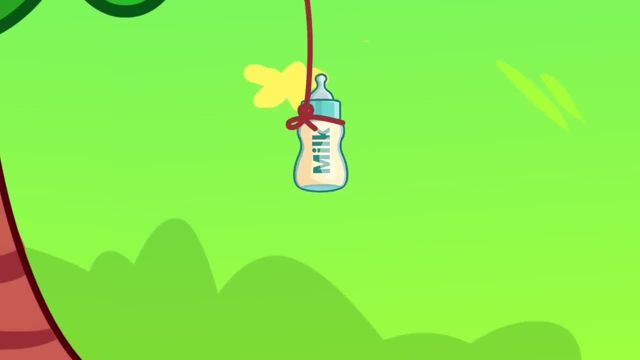 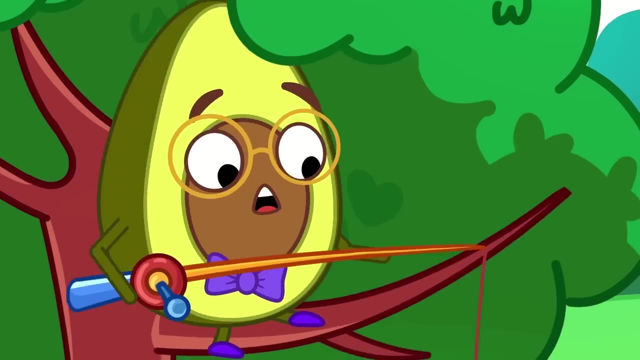 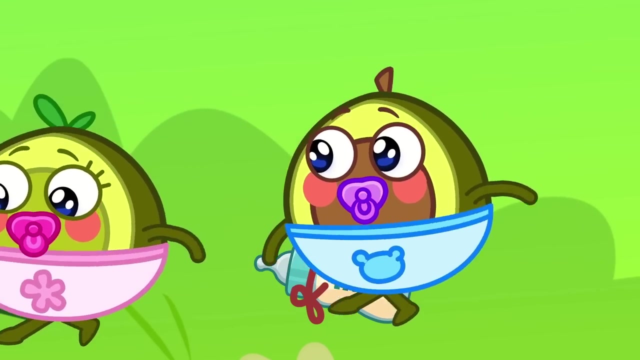 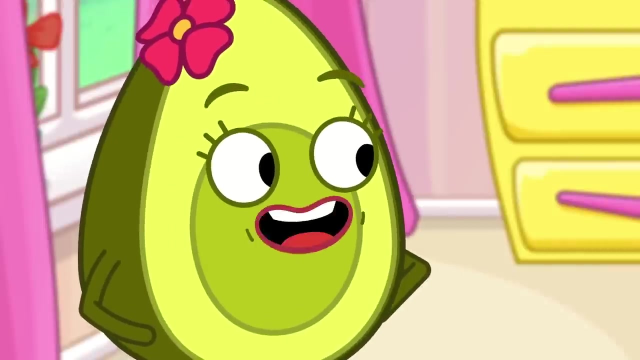 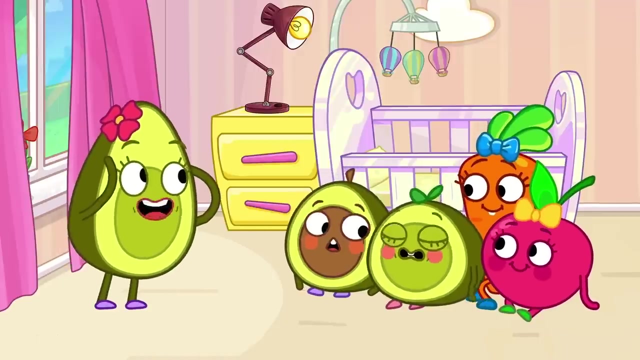 Pit thinks a wrench will work. Do you know how you learn to walk? When Pit and Penny were babies, Daddy used milk on a string to get them to walk. Baby will start walking soon. You have to wait a bit. Where is my baby? 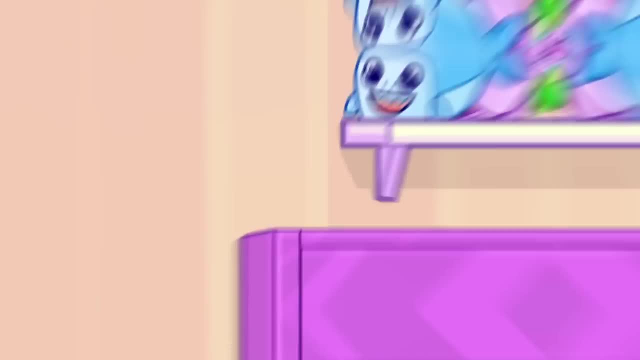 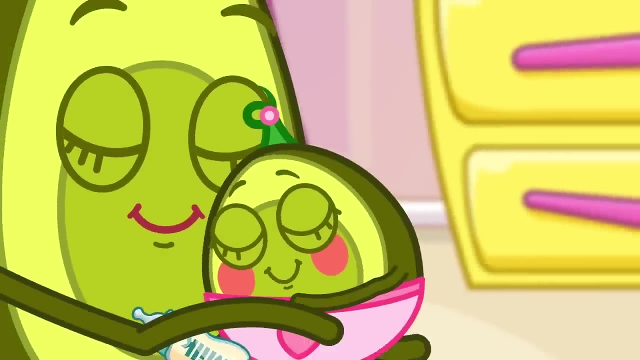 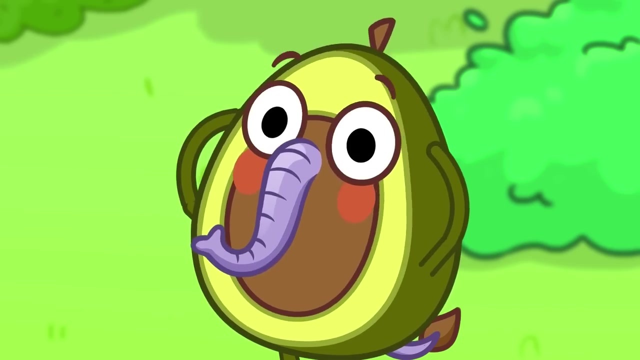 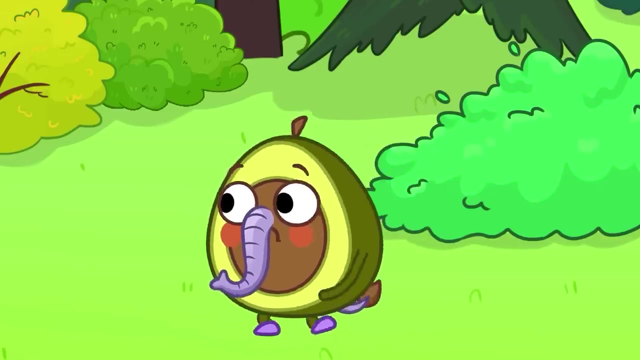 Here she comes And she's already walking. Fantastic job, baby Pit is dressed up like an elephant. What's wrong, Pit? Where are my ears? Oh no, Pit lost his elephant ears. Where could they be? Penny is a bunny. 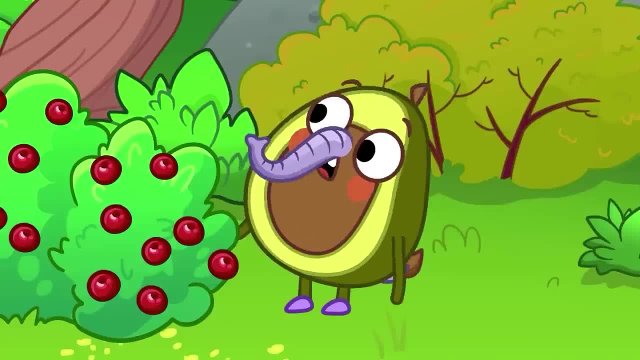 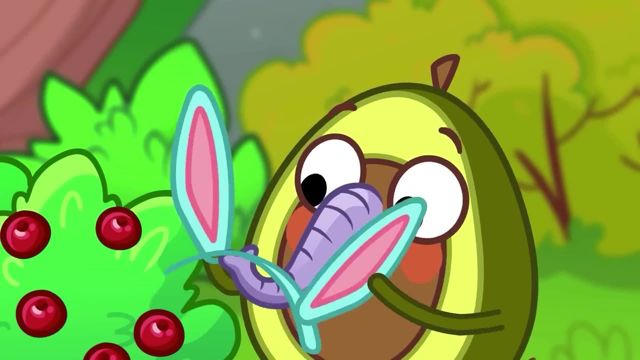 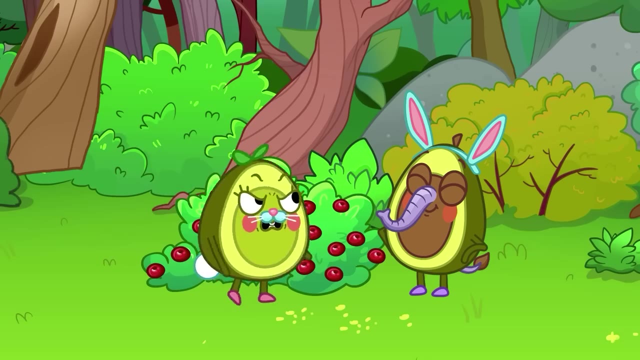 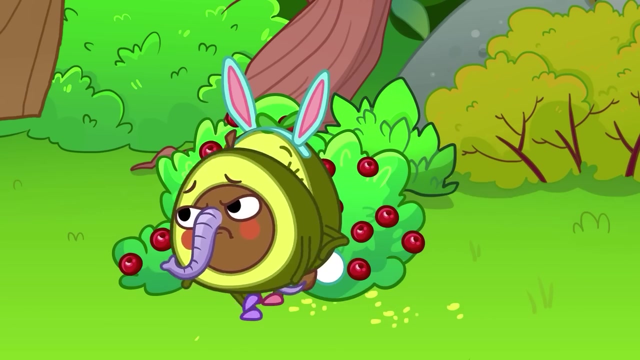 Poor Pit still hasn't found his ears. Could those be Pit's ears? Those are Penny's ears. Penny's ears are so huge and long, but not Pit's ears. And Pet's ears are even bigger. They're like a sheep. 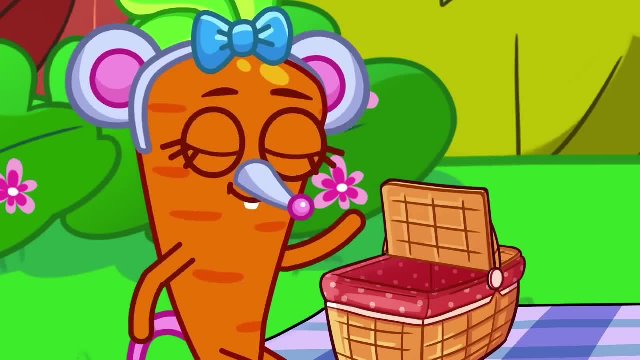 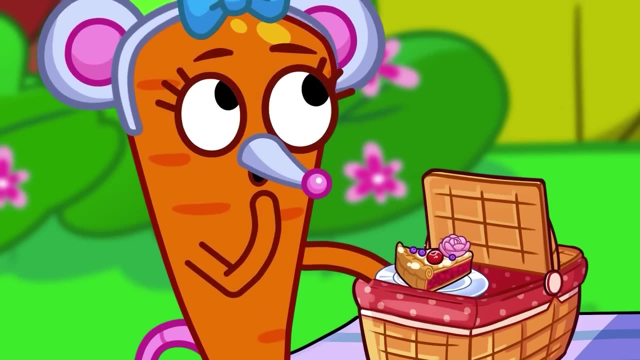 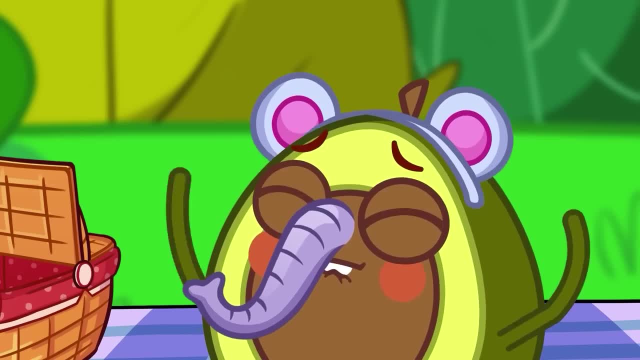 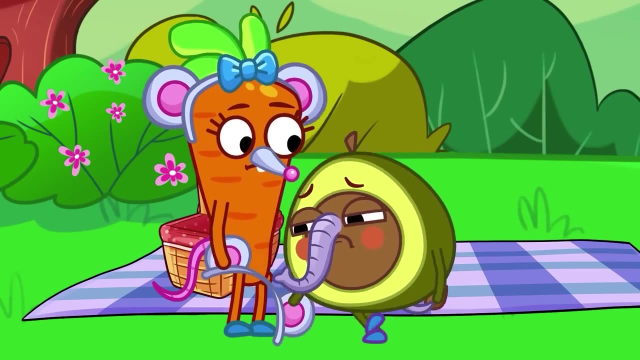 Peek-a-boo, Peek-a-boo, Peek-a-boo, Peek-a-boo. Oh no, Pit fell asleep. Pit fell asleep. Yeah, Pit fell asleep. Pit will have to keep looking. Cherry's a cat, The wind took her ears. 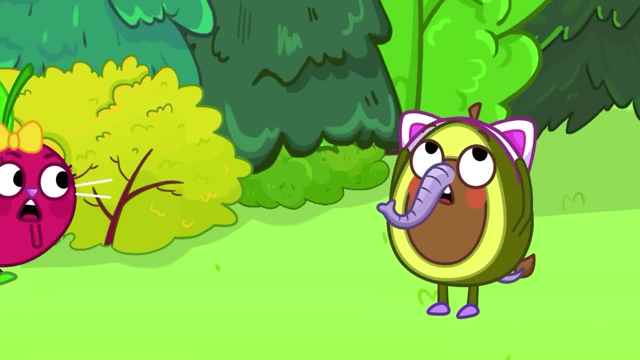 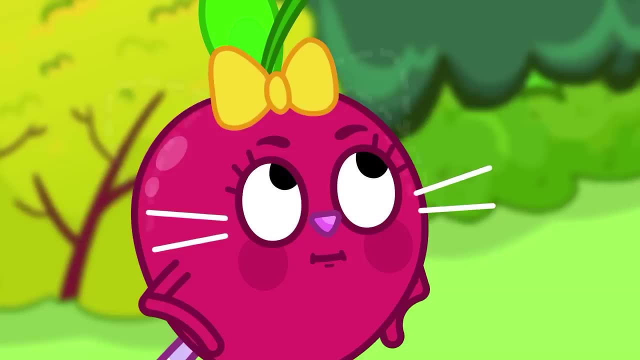 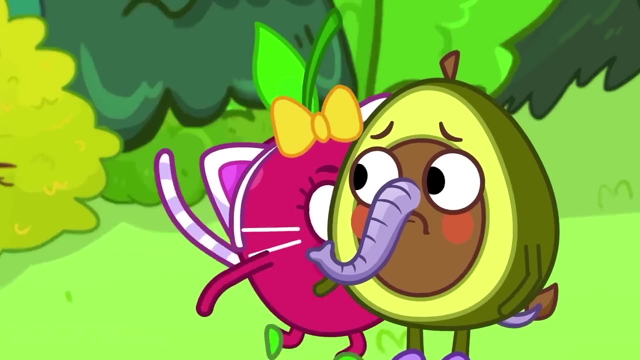 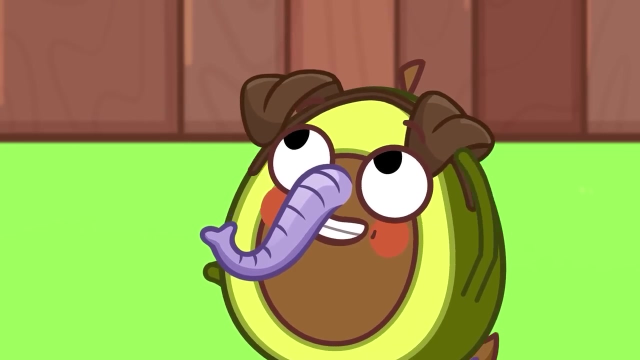 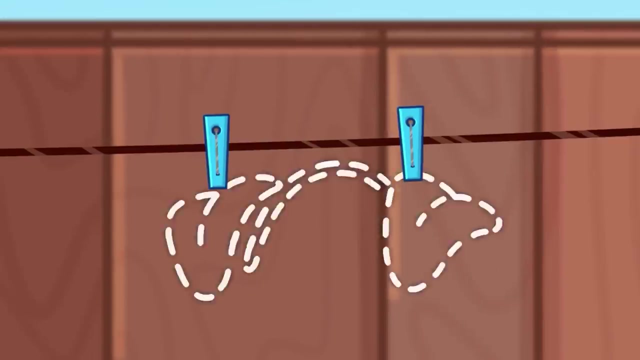 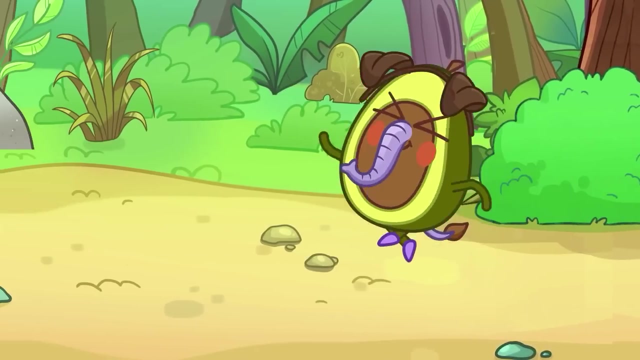 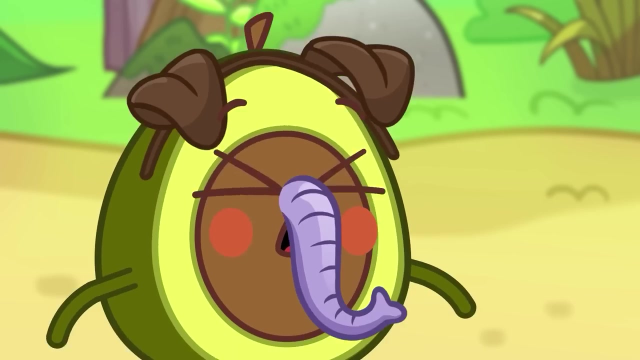 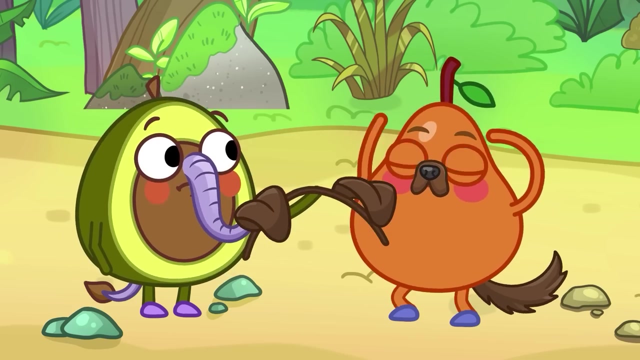 Are those Pit's ears? No, they're the ears Cherry lost. There are some ears, But are they the right ears for an elephant? Those ears belong to Pear the dog Pit. you're wearing Pear's ears. I've lost my ears. 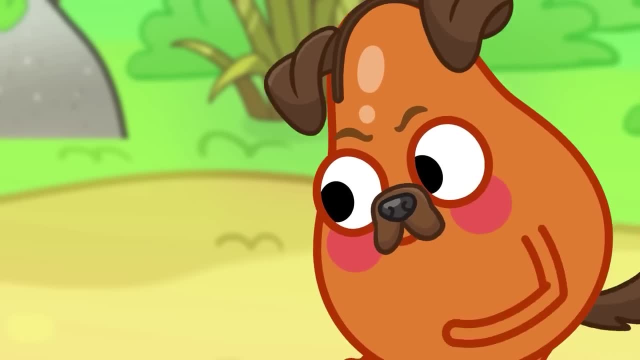 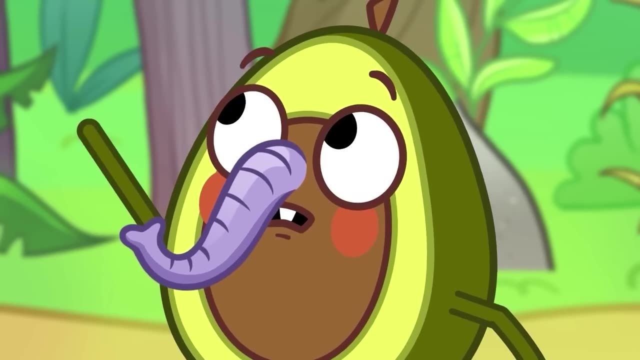 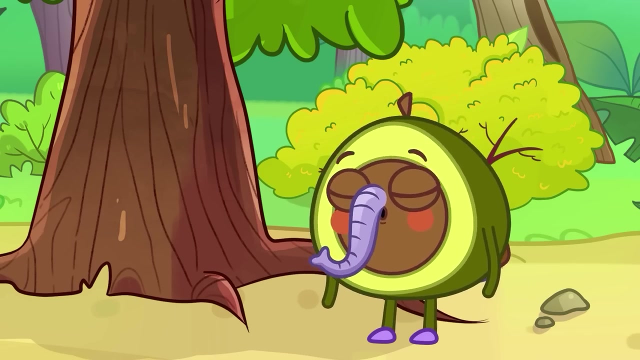 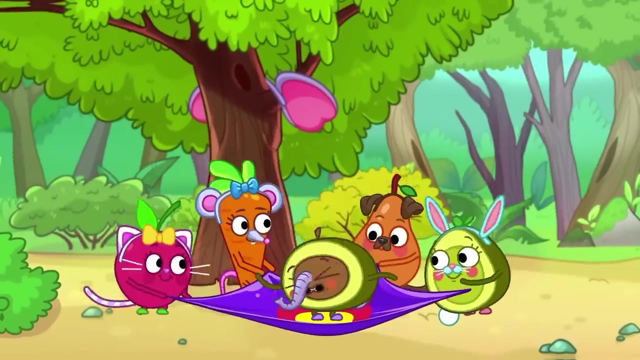 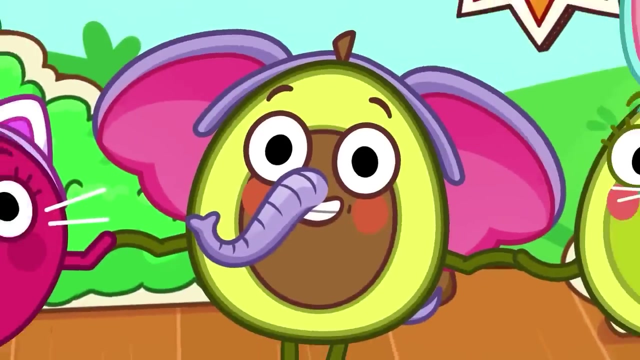 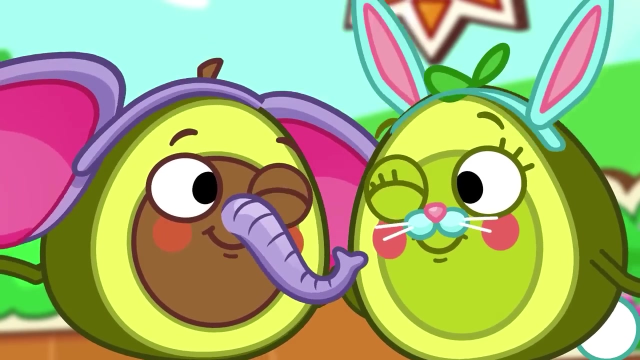 Maybe Pear can help find them. It's the elephant ears, But they're too high to reach. We will help you A little higher. You did it, Pit. Hey, Friendship helps in trouble. What a wonderful play. Pit and Penny made a cardboard fort. 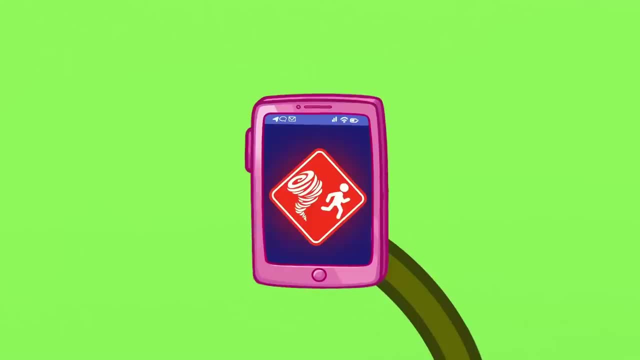 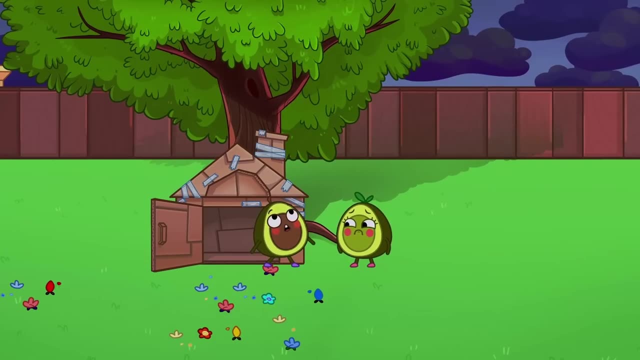 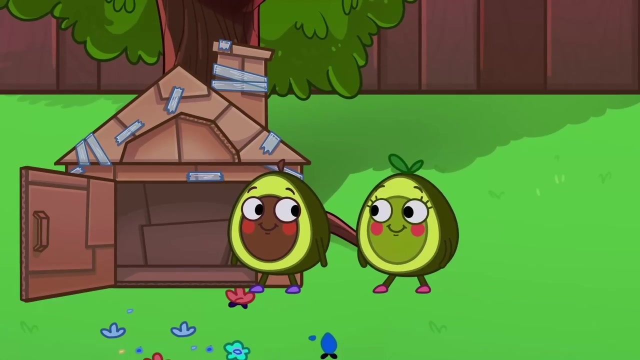 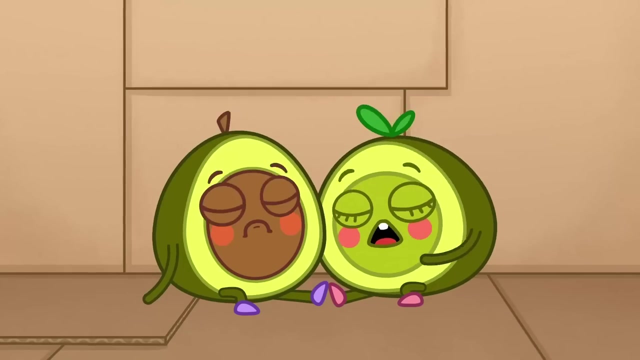 What? What is it? Penny? It's a weather warning. Oh no, Hurricane Run. You better get inside the house. Our fortress will be safer. The storm sounds very strong. There you are, Quickly get into the house. 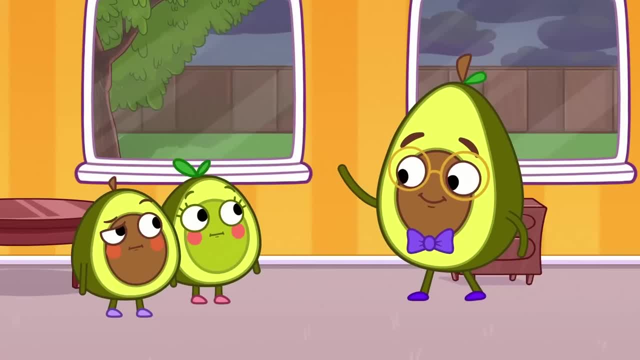 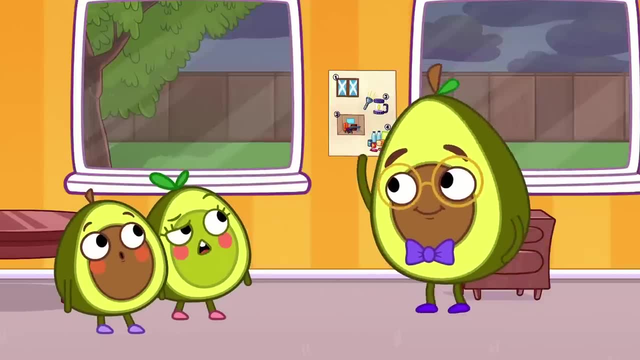 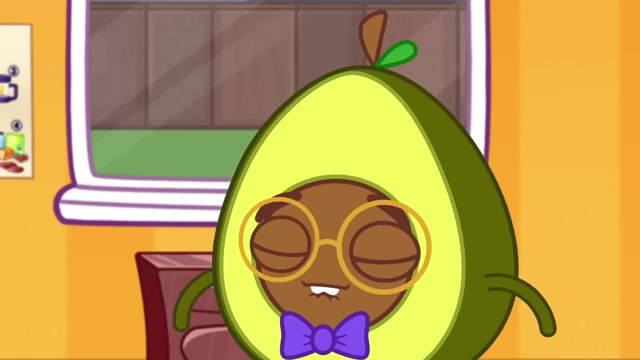 Let's go, We will be ready for tomorrow. Come on, Go, go, daddy. Come with me. Daddy has a special checklist to keep everyone safe. Will you help us get ready for the storm? What should they do first, daddy? 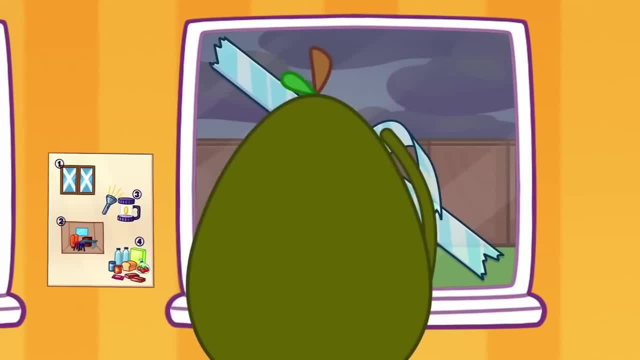 First put strong tape on the windows. Penny made a snowflake. He came to the window to get some air. I thought I'd have to draw really fast before doing this. I have no idea what to do. I don't know. 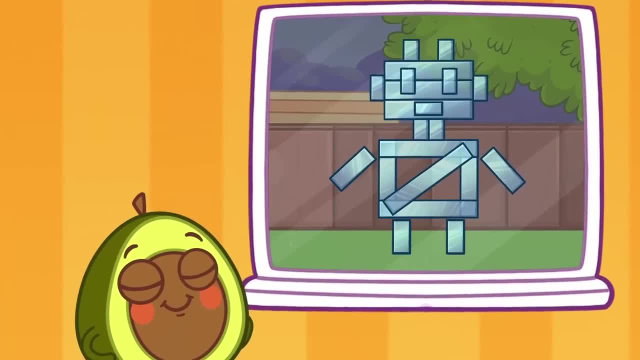 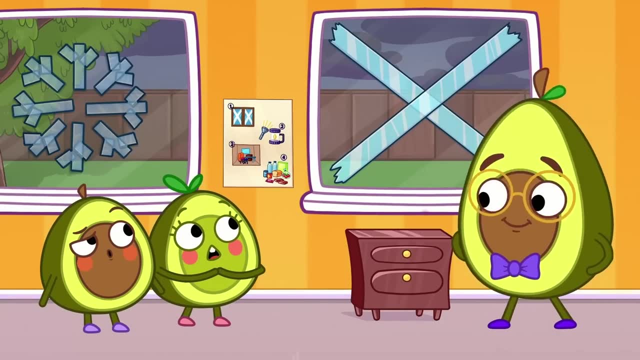 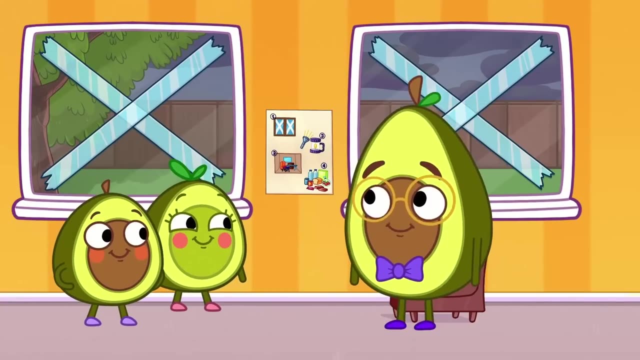 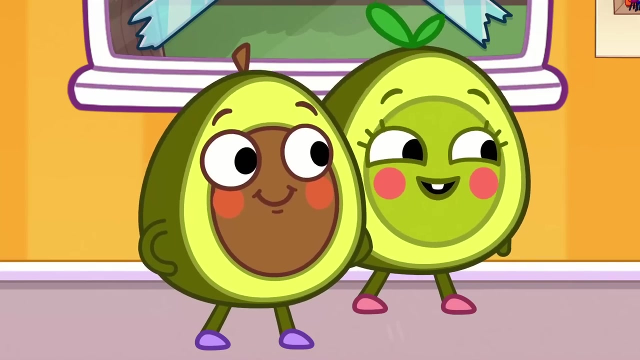 You know what to do? I don't know. Come on, come on on, Come on, come on. plate Pit made a robot. The windows have to be sealed diagonally with duct tape. That's much better. kids, What's next? Move everything away from the windows. That couch is very 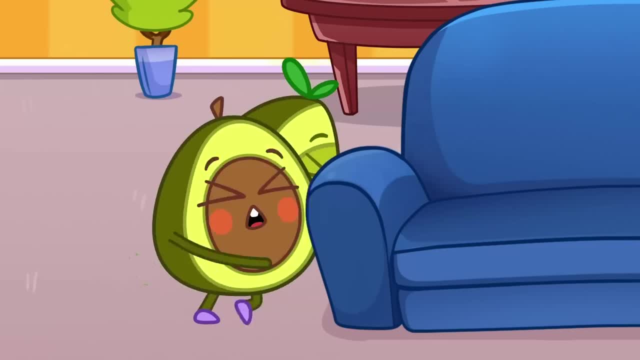 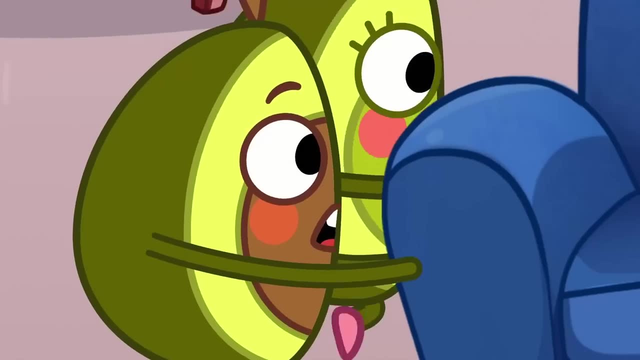 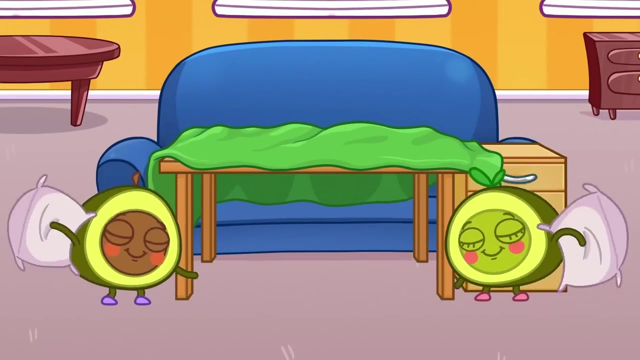 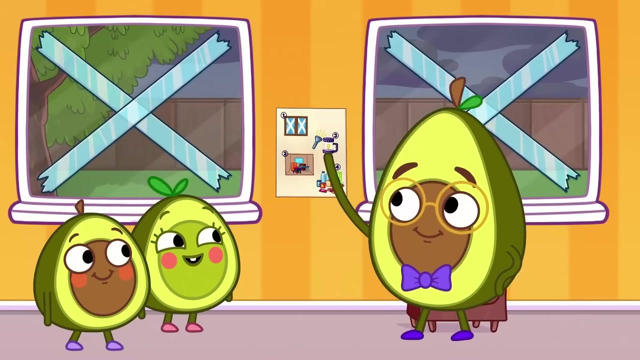 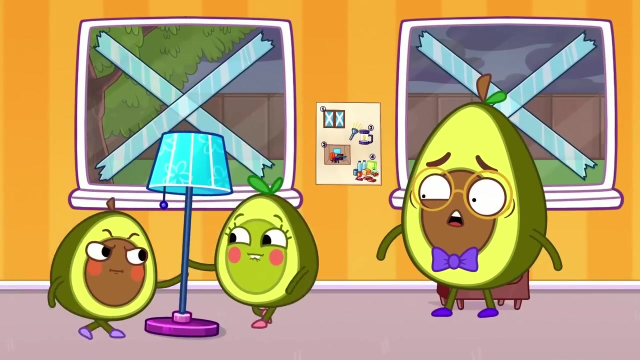 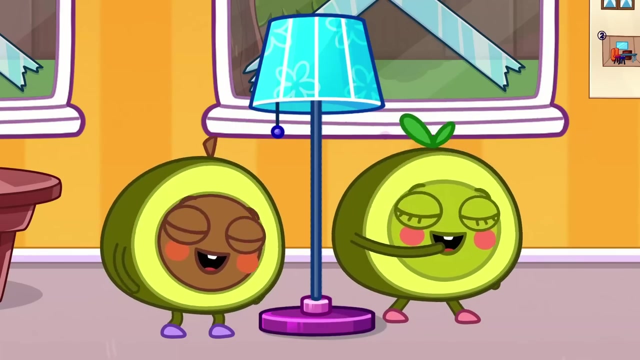 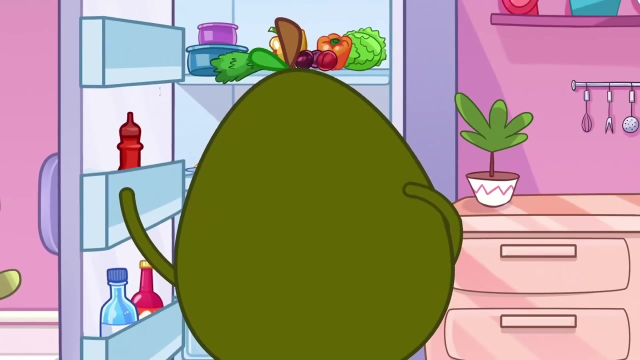 heavy. Oh pit. Time for step three. Now we need a backup light source. Will this lamp work? We have enough flashlights. And don't forget about food. What can Pit and Penny find in the kitchen? They found cake. It's better to choose something that. 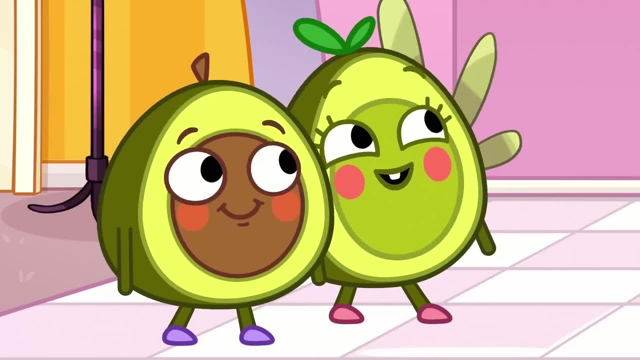 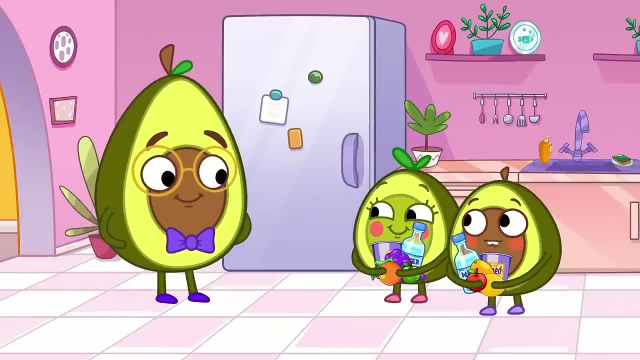 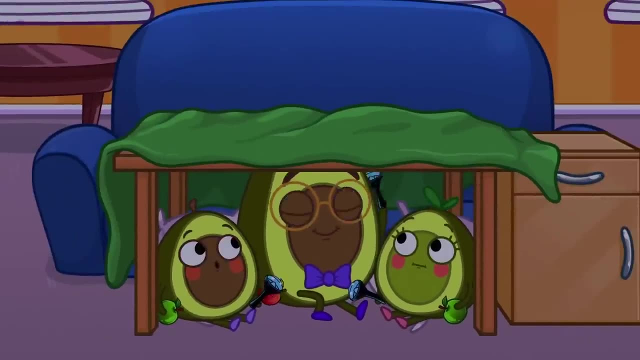 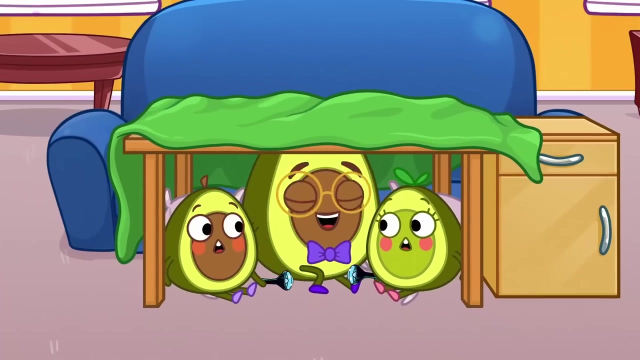 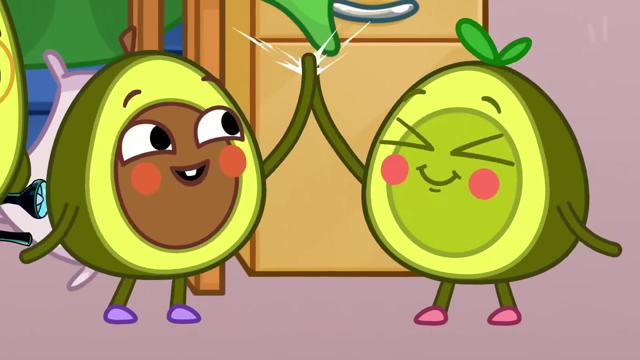 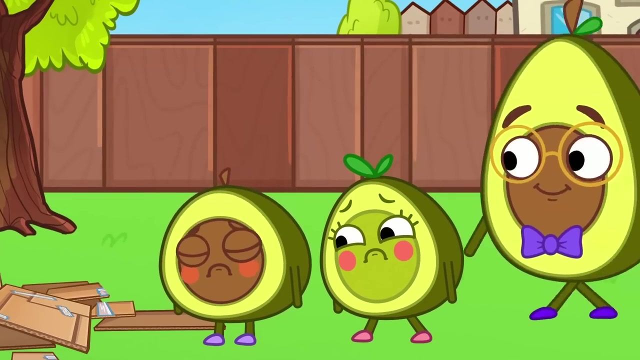 will not go bad for a long time. Bottled water and fruit are perfect. Hopefully, the storm will end soon. Hooray, You've handled the storm very well. Now you can play in the fort. Oh, the fort was blown down in the storm. 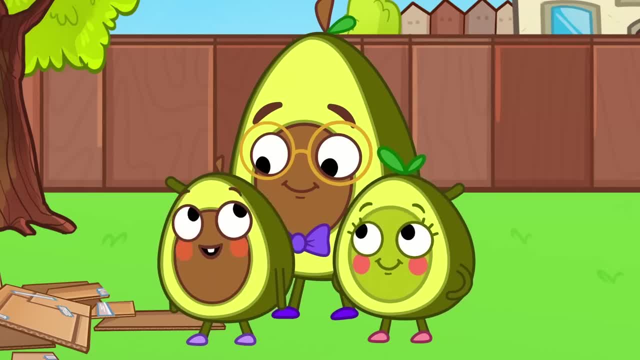 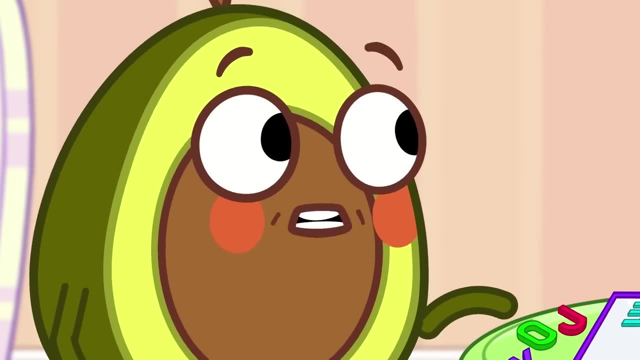 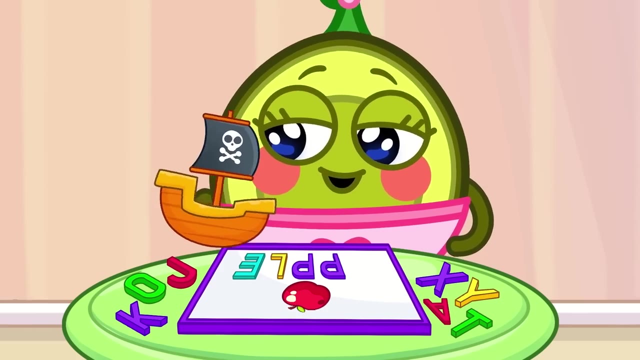 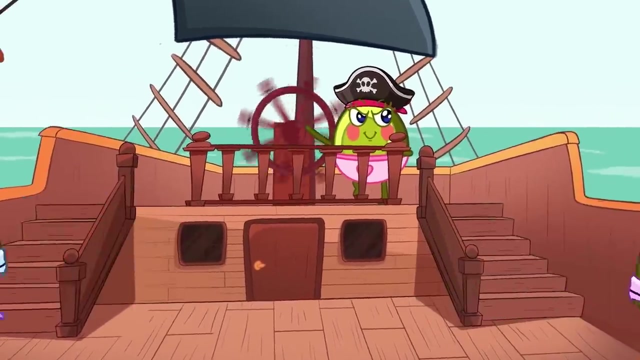 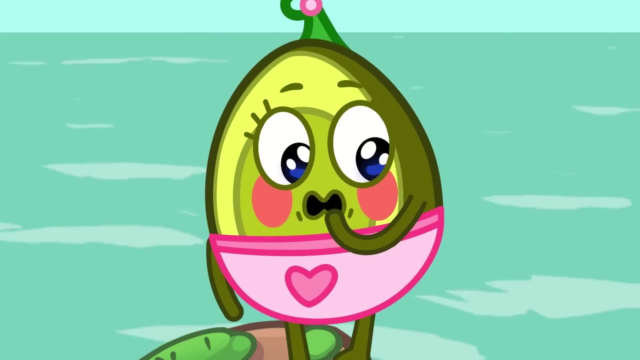 You can't hide from a hurricane. outside, Pit and Penny are teaching Baby the alphabet. Baby just wants to play. Now she's dreaming she's a pirate captain. Oh no, She's been blown out to sea And the ship is so far away. 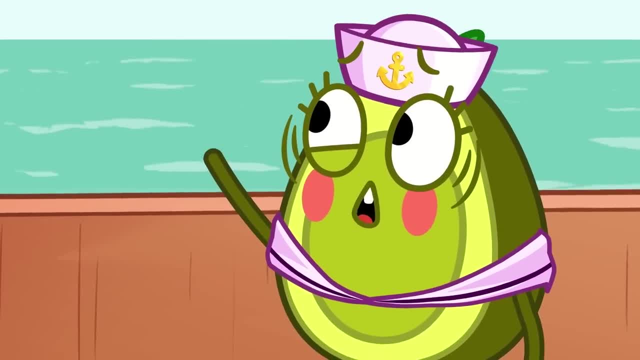 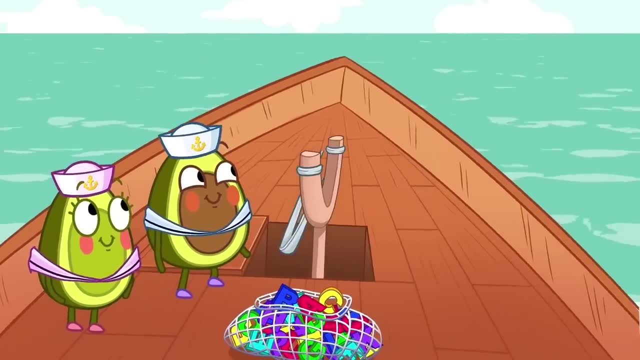 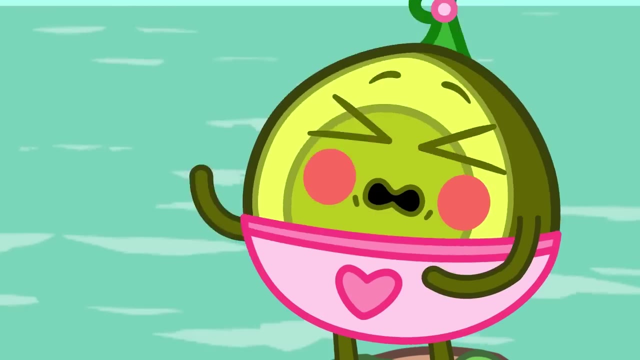 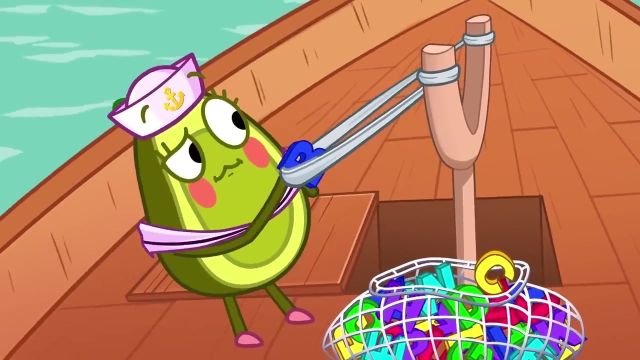 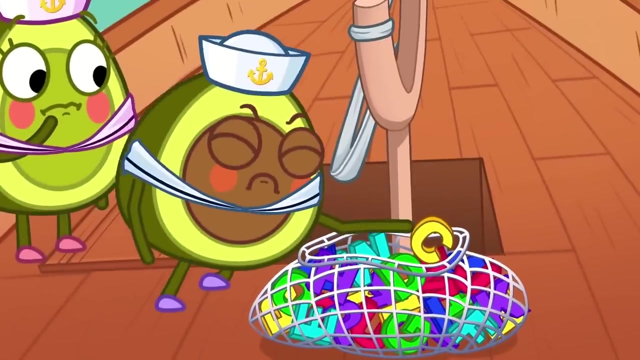 Oh no, We can't steer the ship without a captain. But how will you save her? These magic letters will help. A for apple: Hop on the apple baby. B for banana: The banana didn't go far enough. C for cake: 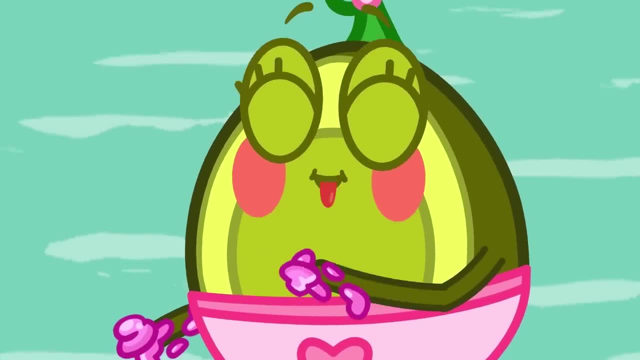 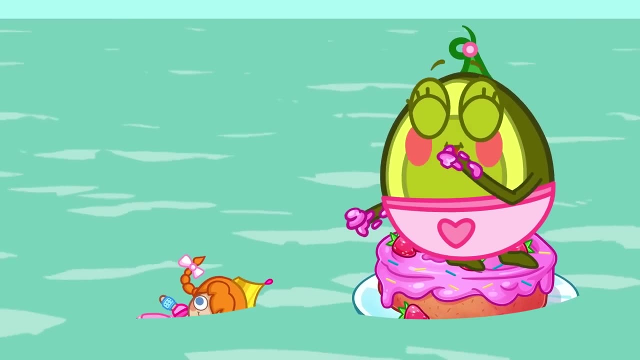 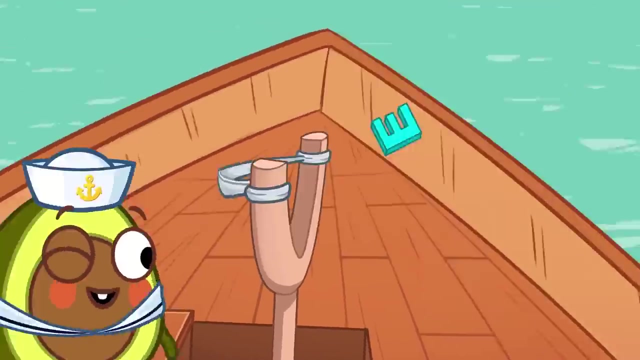 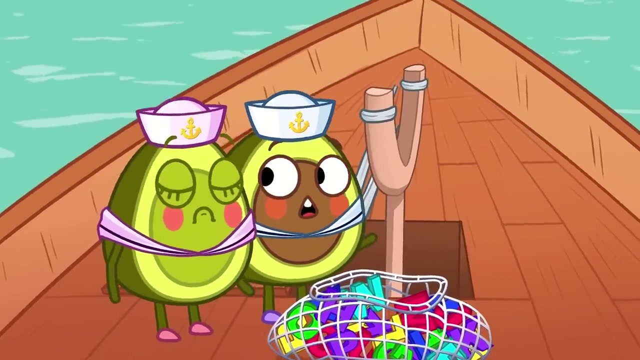 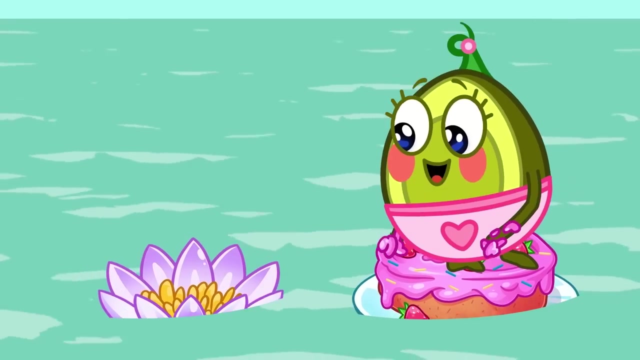 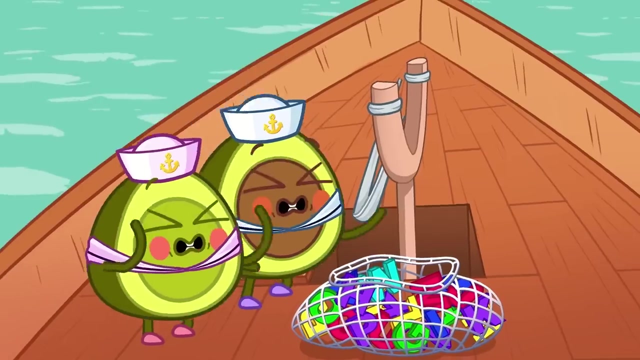 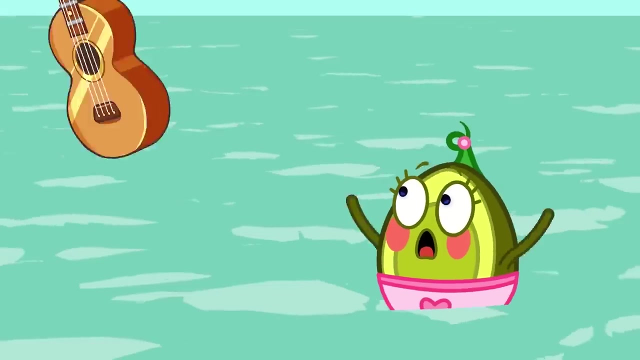 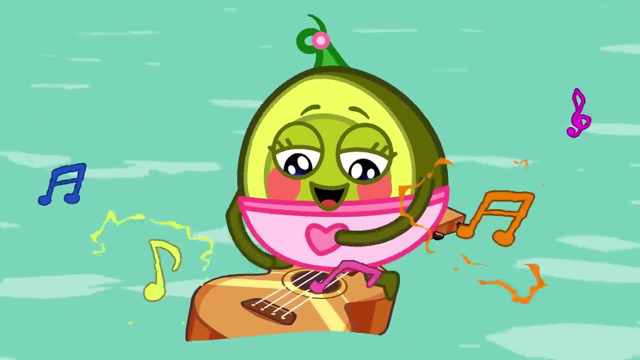 Yum. Z for dog: Uh-oh, Baby's too busy eating. Try something different. E for eagle: The eagle flew away. F for blower, But the flower is sinking. G for guitar: Phew, Now baby is safe. 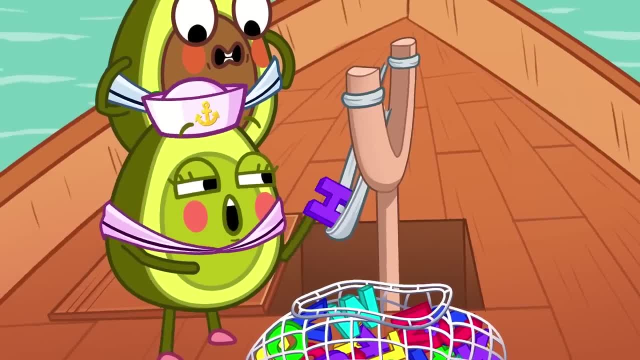 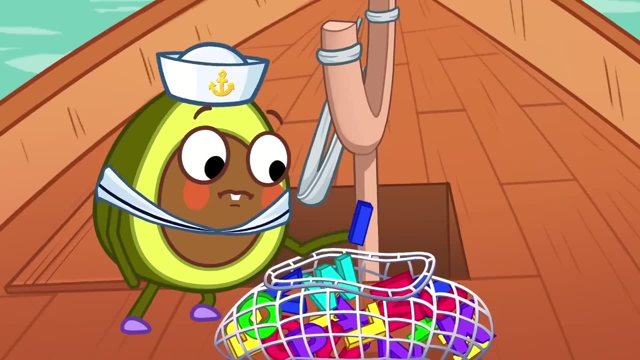 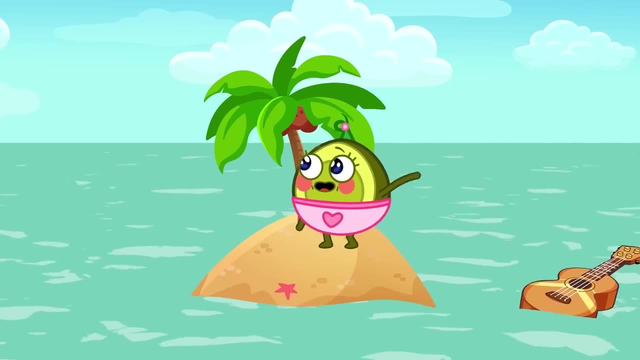 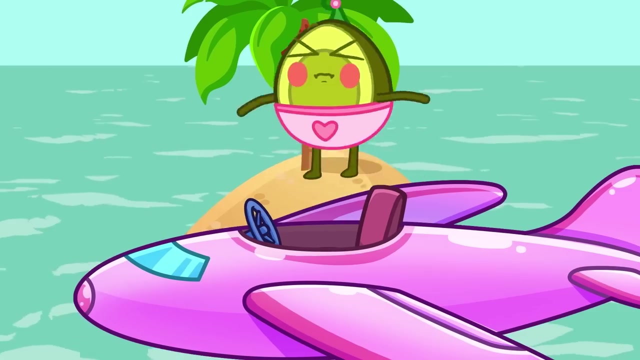 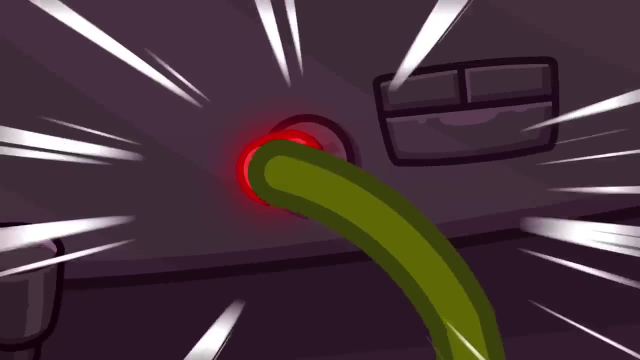 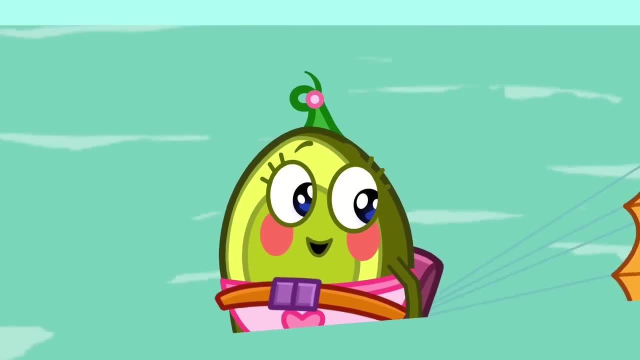 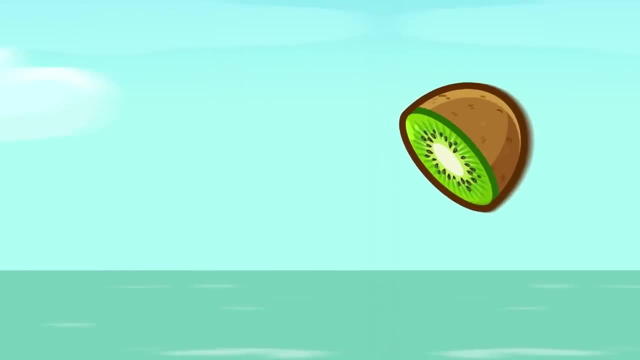 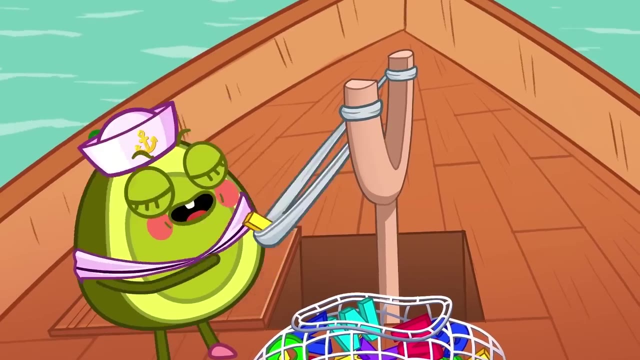 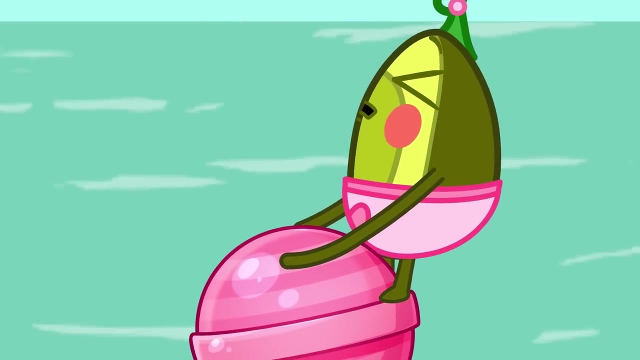 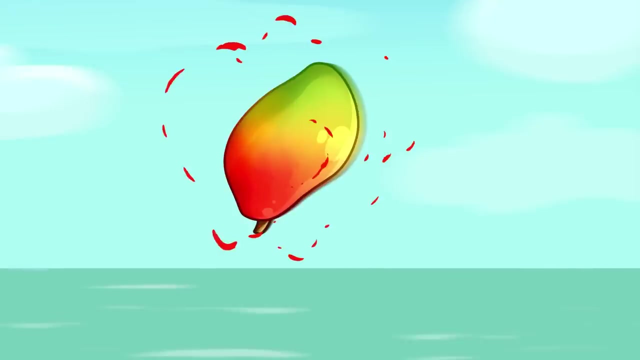 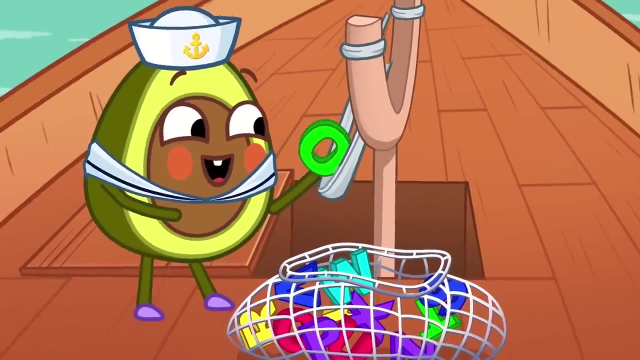 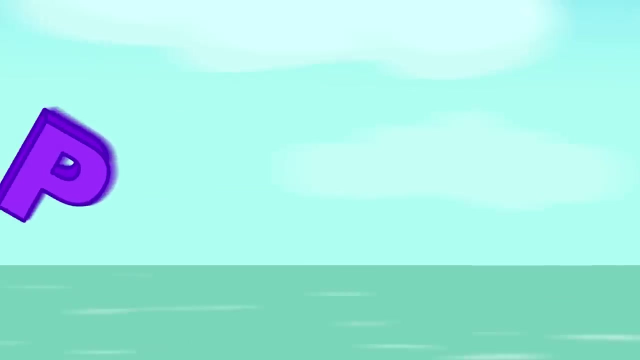 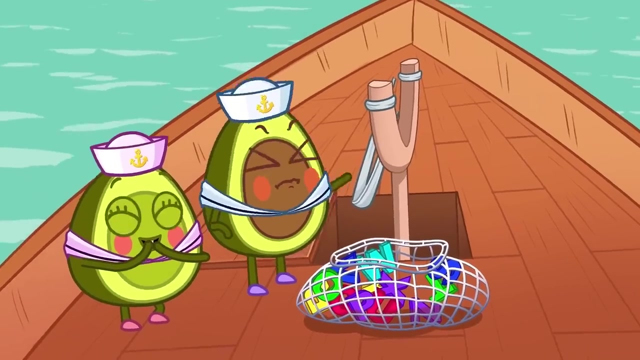 K for kiwi: Baby's gonna fall in. And for mango: Careful, you almost hit Baby. Oh for Onion. Baby for Pineapple. You for Quill. The Feather made Baby sneeze. R for Rattle. 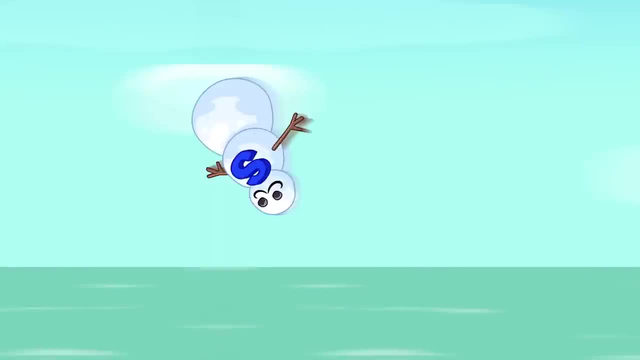 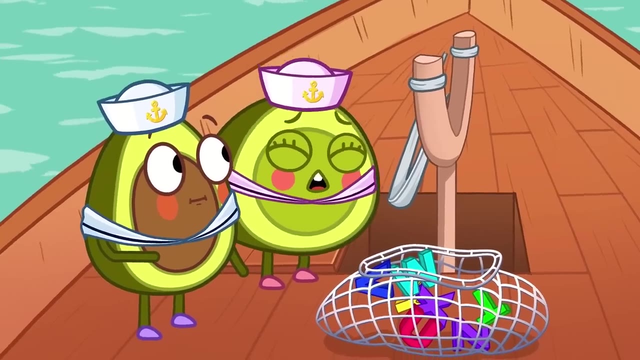 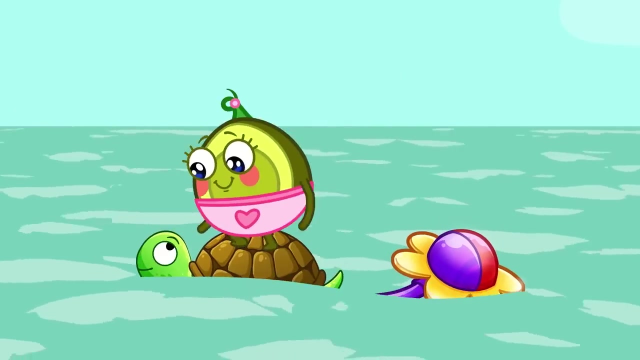 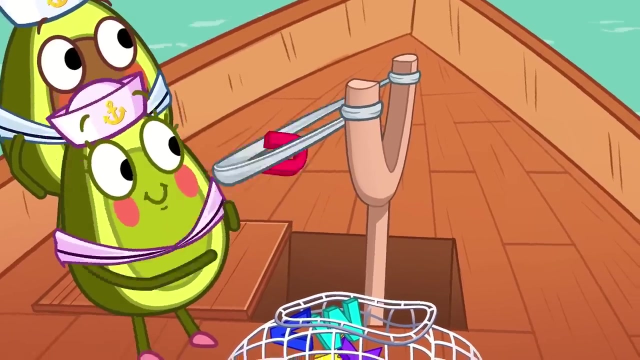 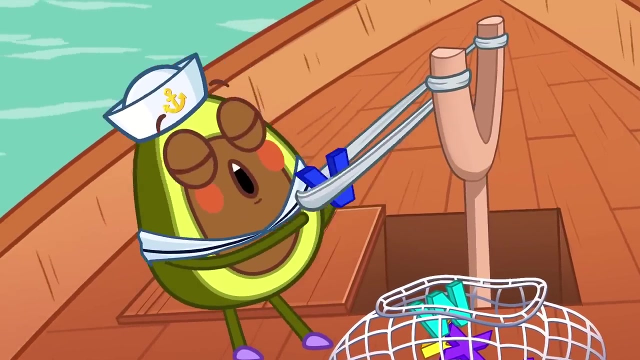 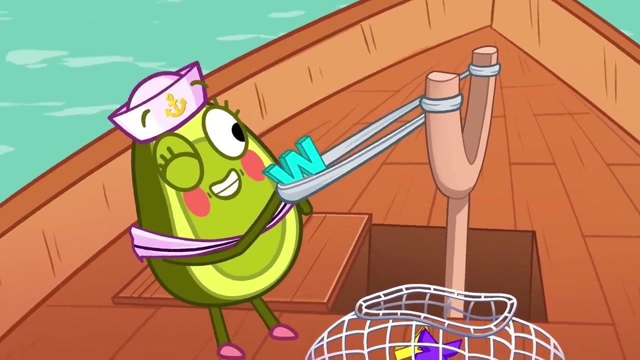 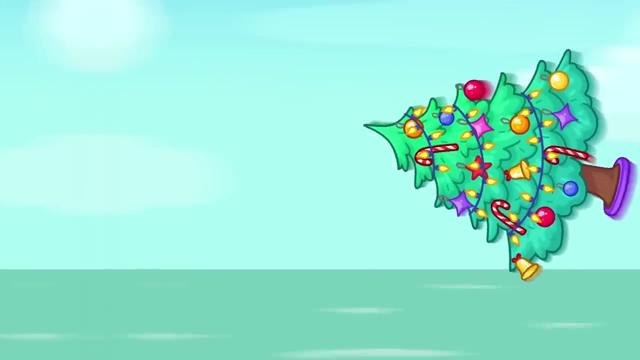 S for Snowman, The Sun melted. the Snowman. T for Turtle: Baby is almost at the ship. U for Umbrella. V for Volleyball. W for Watch. X for Christmas: The Splash pushed Baby further away. 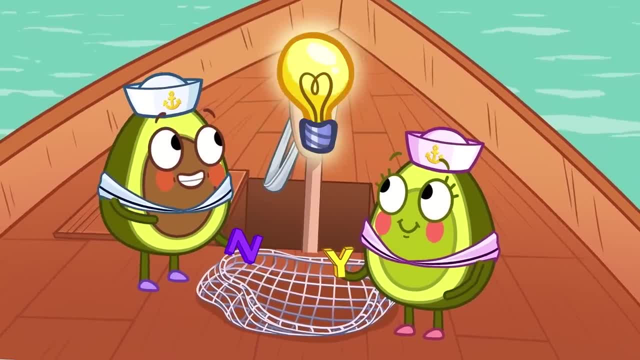 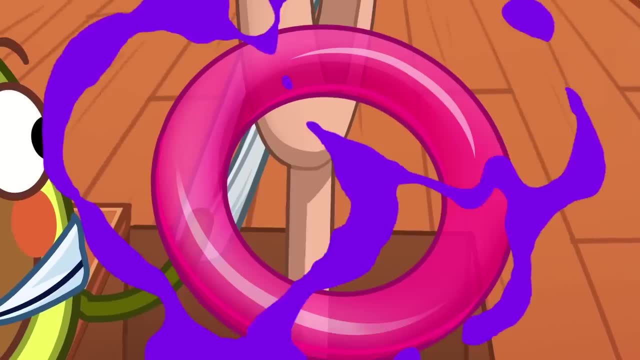 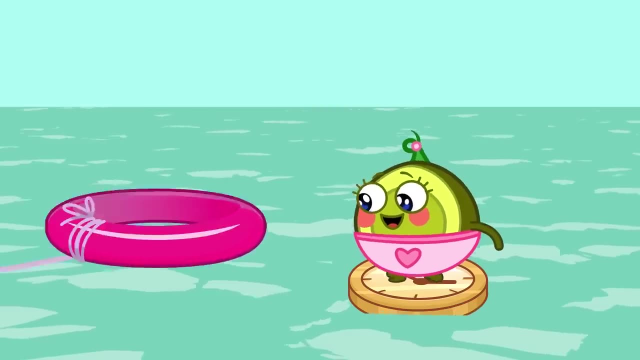 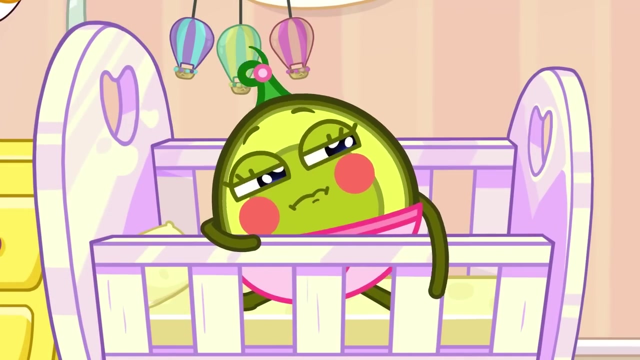 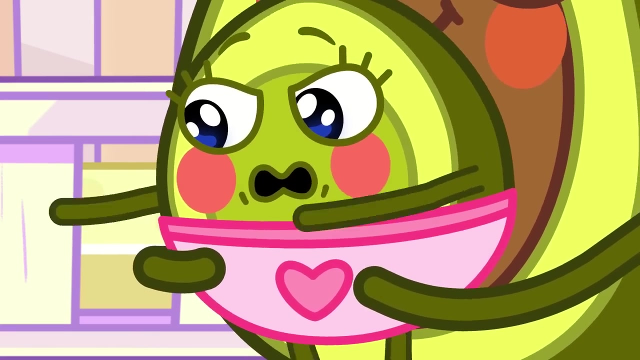 Try to work together. Y my yarn, Z for Zero. Now throw it to Baby. See, She's safe and sound. Her Sheep sews baseball on the shore. Daddy's shoes. Raise the ball, Bend the ball and make it go. 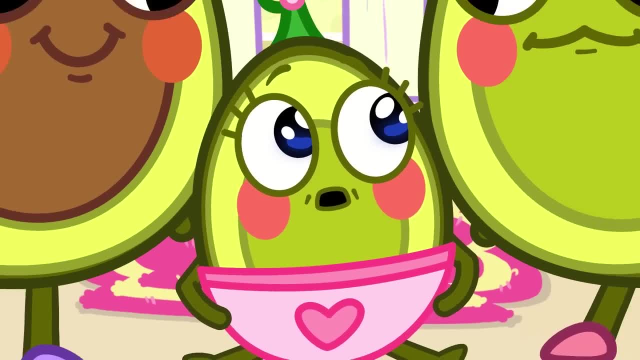 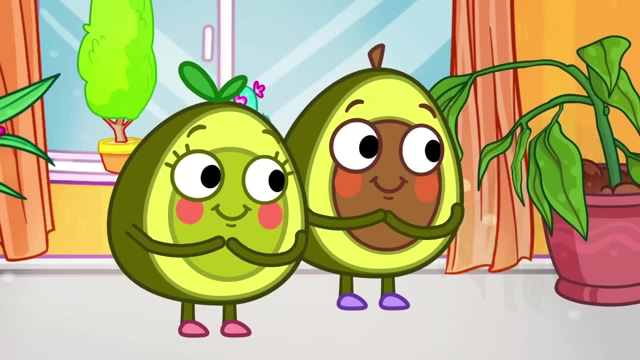 Take the ball to the mound where she passes. ודuded- Dodip is next Swing. do your best. Everything's counterclockwise. R for Union. Oh, what a affect. What is it, baby? R for Apple. 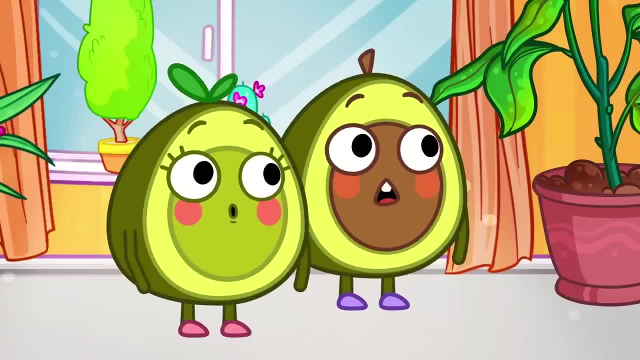 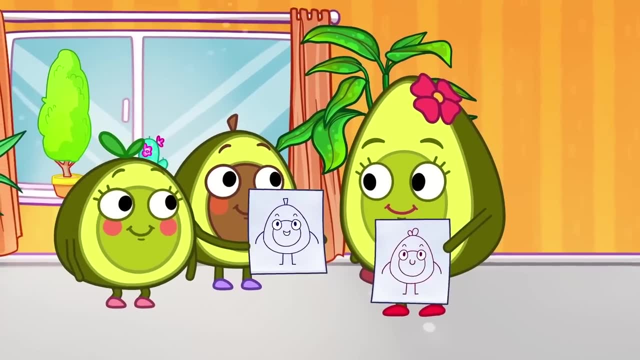 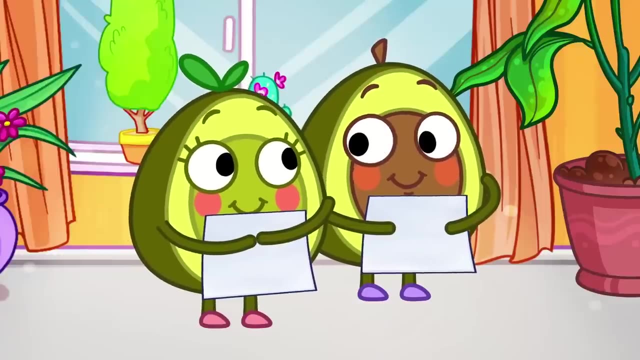 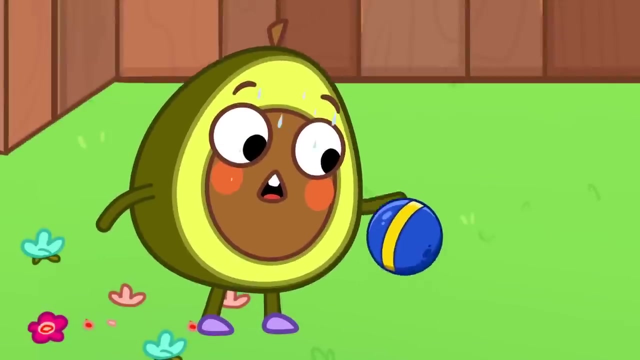 Well done, Girl startups- Up to 3 positions- Good job. Color these pictures blue every time you drink water. This will help you keep track of the water balance in your body. Pit's playing outside with his ball, But he's getting very hot. 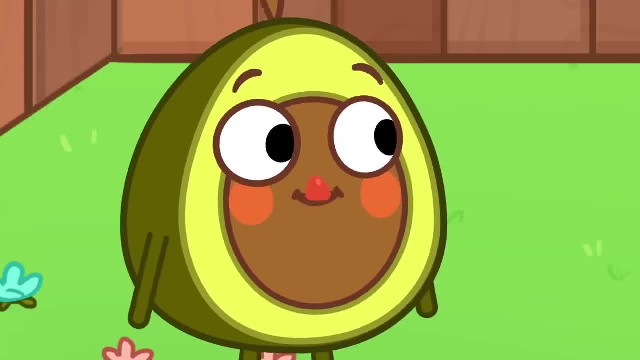 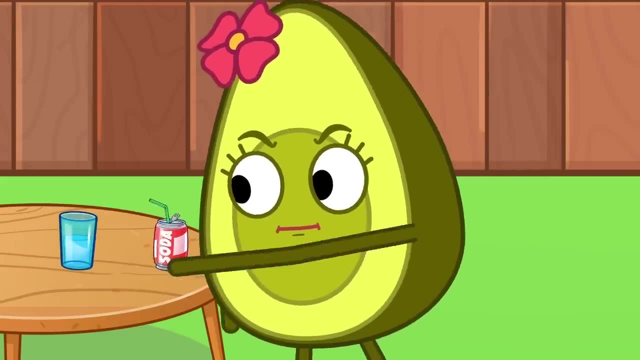 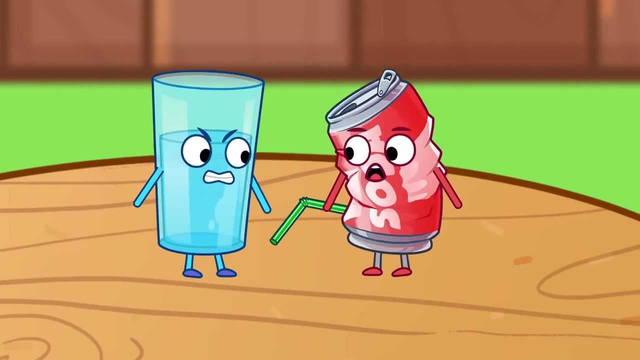 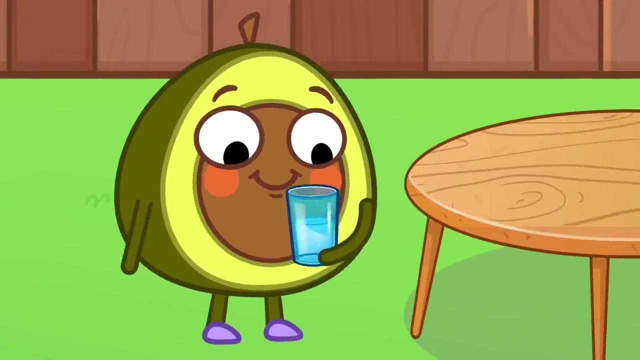 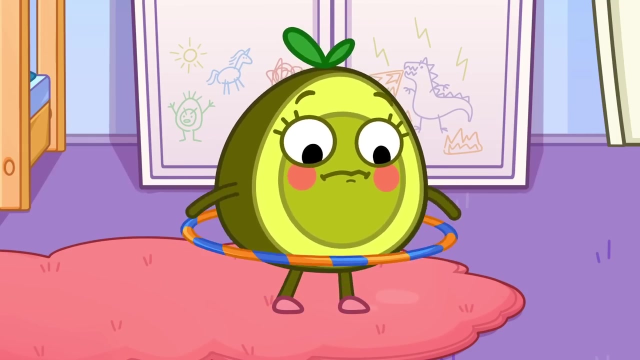 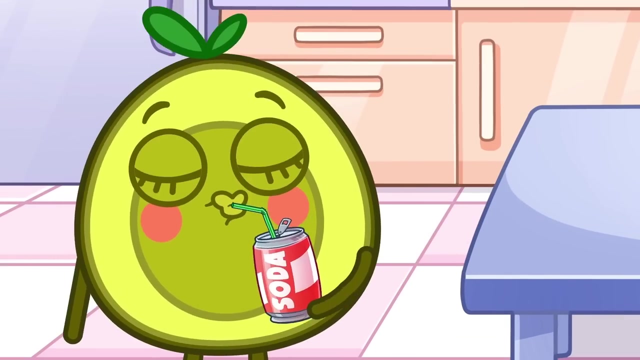 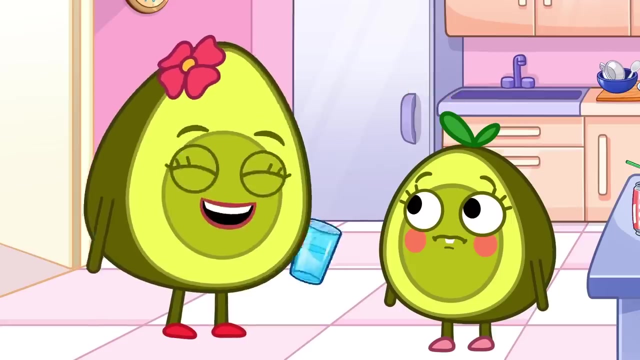 He wants some soda. Soda is not water. Water is a better choice. Try it. Pit. Penny's playing with her hula hoop, But now she's thirsty. Penny, you shouldn't drink a lot of soda. Water will help you. 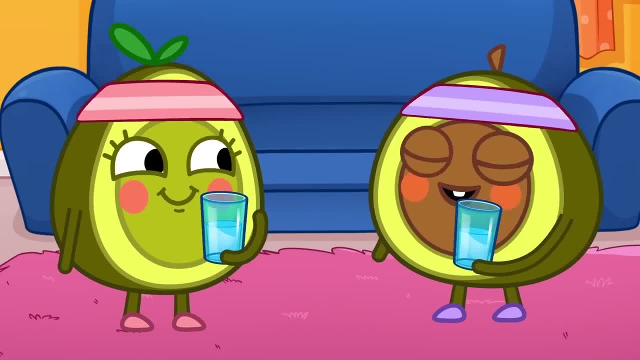 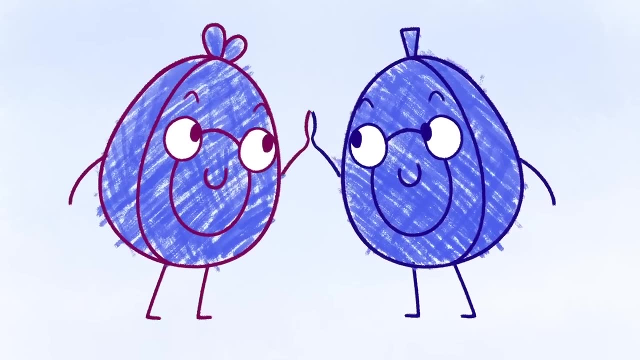 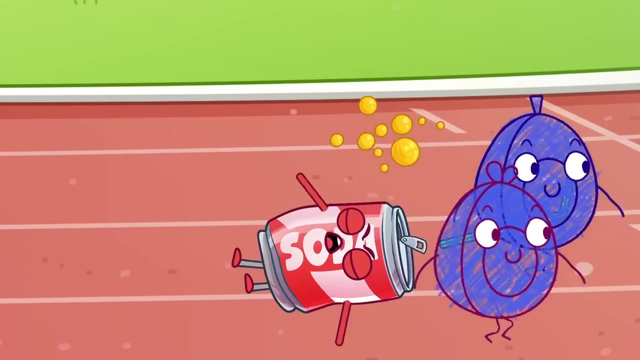 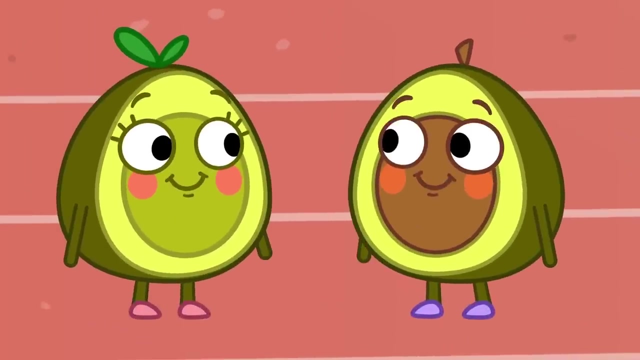 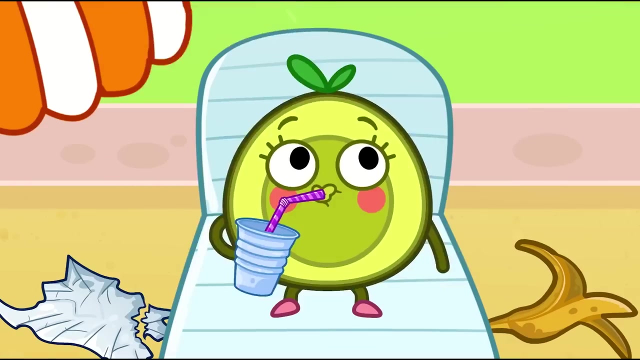 Water will give you energy. Hit him, Penny. I drank lots of water today. Sorry, Soda, You're not as good as water. Well done, Pit and Penny. Pit and Penny are at the beach. Everyone's having fun, Wee. 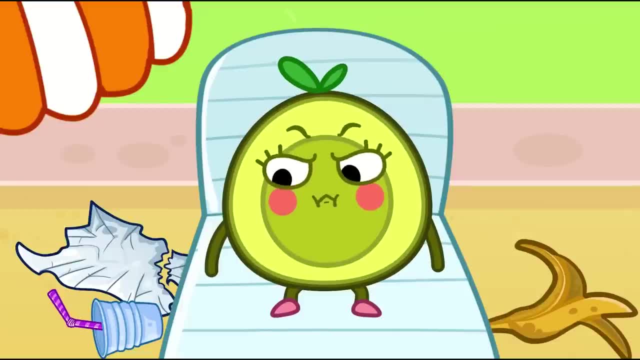 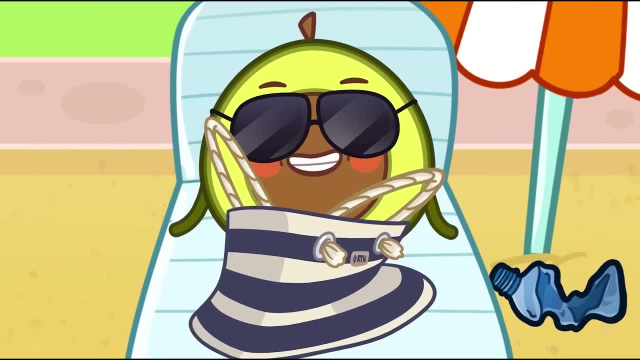 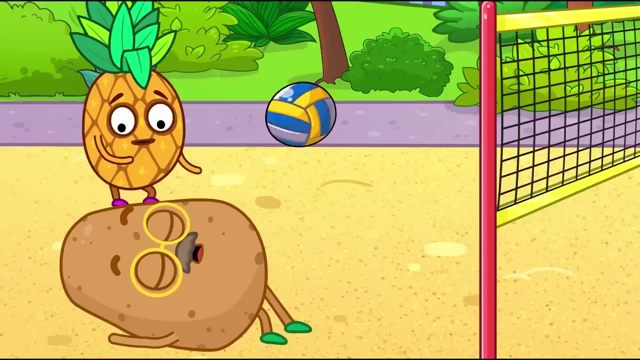 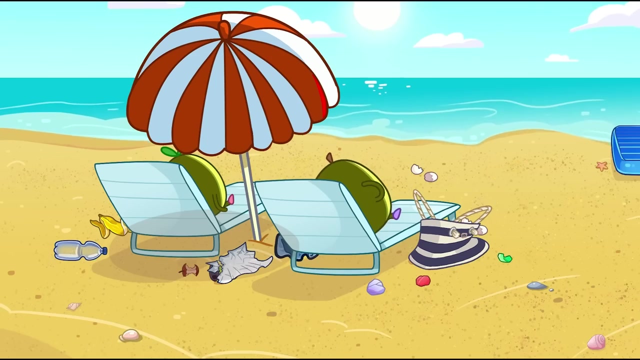 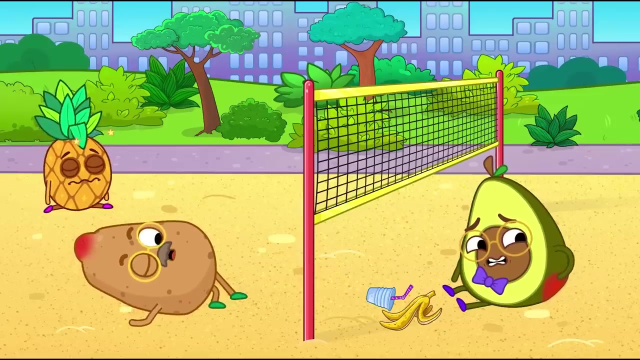 Poor Penny. But Penny… That's literal, And so is that. Watch out, Dad. Oops, Penny and Pit are leaving garbage everywhere. Everyone's hurt, And it's because of Penny, It's all because of the litter Time to clean it up. 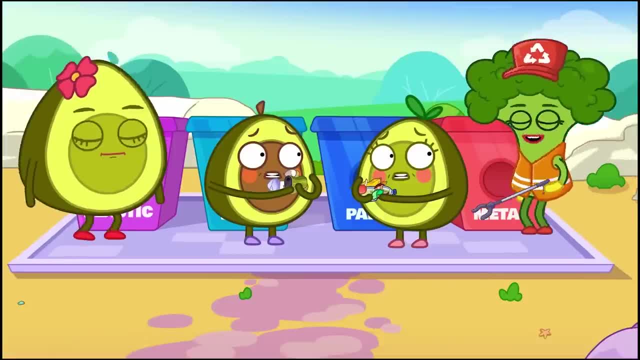 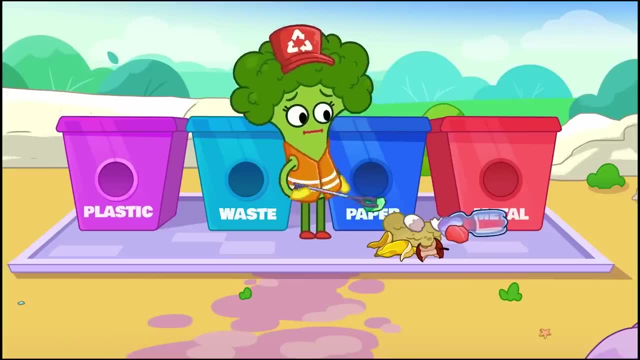 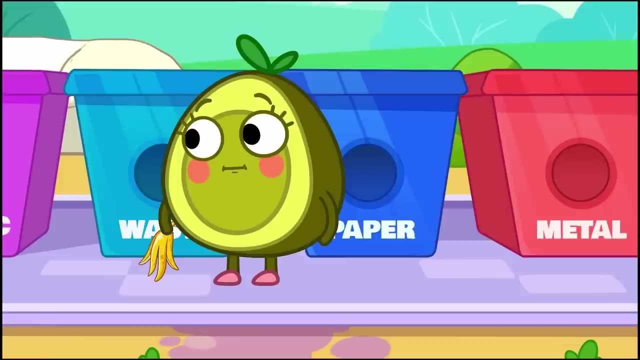 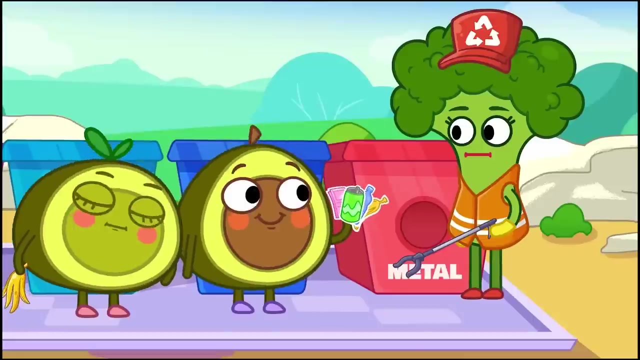 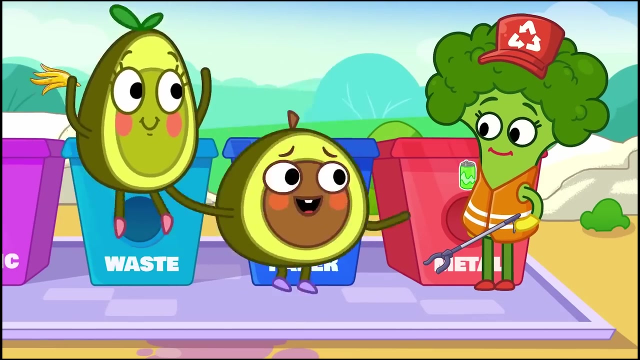 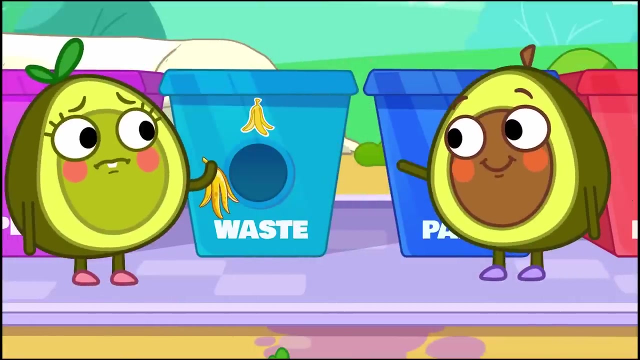 Stop. It's a paper bin. If you put it all in one bin it makes more work for her Place each item in the correct bin. Pit's stickers will help. Plastic waste, paper and metal. Hmm, where does the banana peel go? 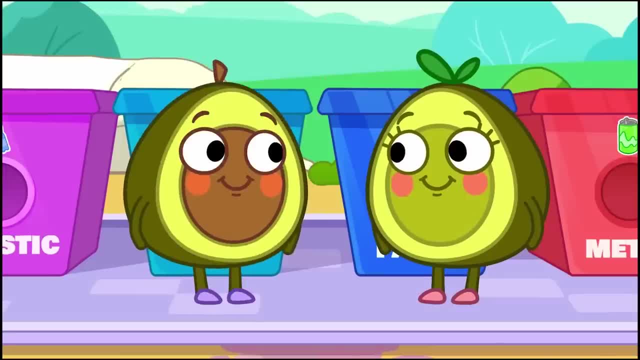 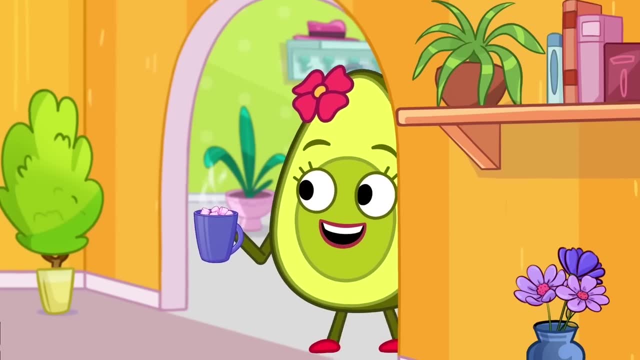 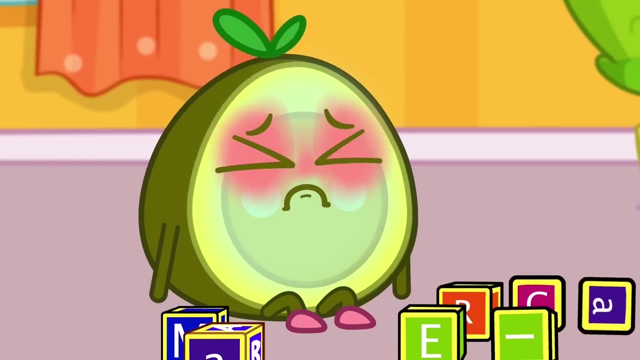 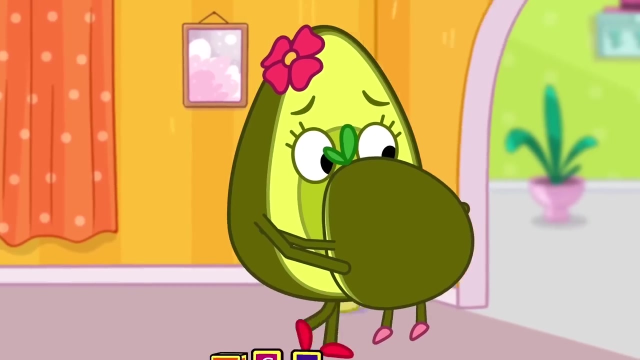 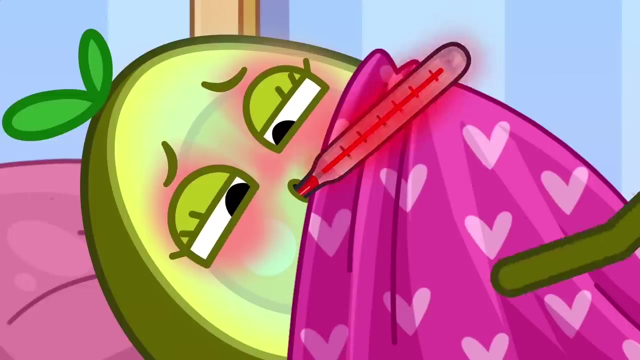 Good job, Pit. Now everyone can enjoy the beach. Mommy has made a delicious cup of coca. Oh no, Penny is sick, Dear, You've caught a cold. Mommy puts Penny to bed and makes her cozy. That doesn't look too good. 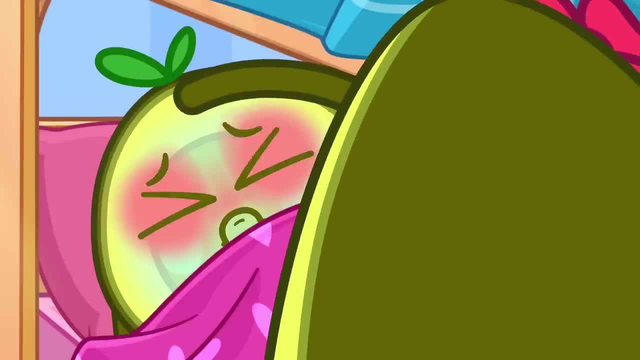 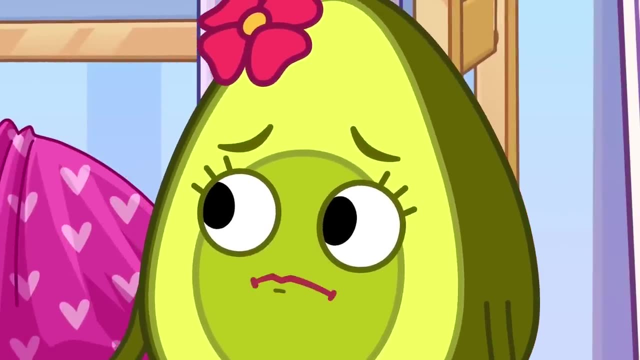 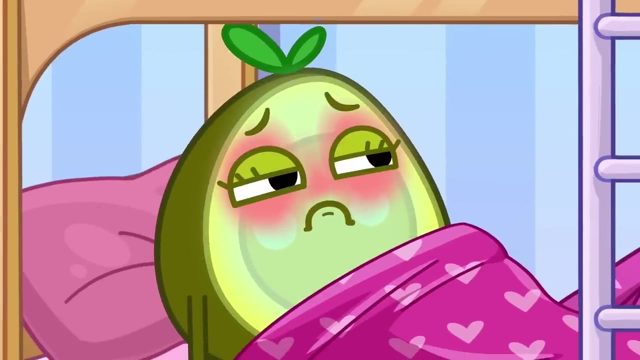 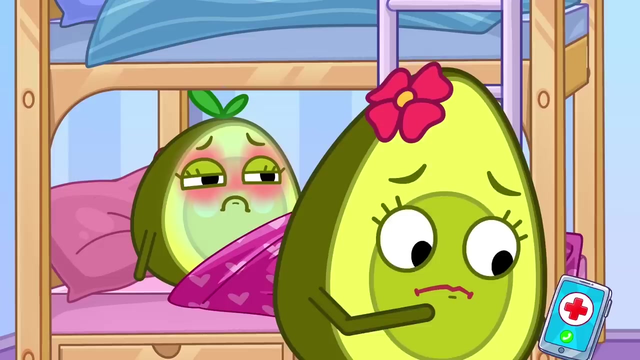 Maybe the thermometer is broken. Penny is feeling hot. You have a fever. I'm calling a doctor. No, I don't wanna, But Mommy is worried, so she calls the doctor. Penny is not happy. Someone is at the door. 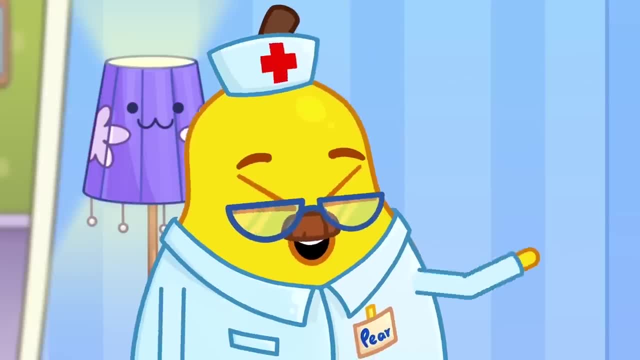 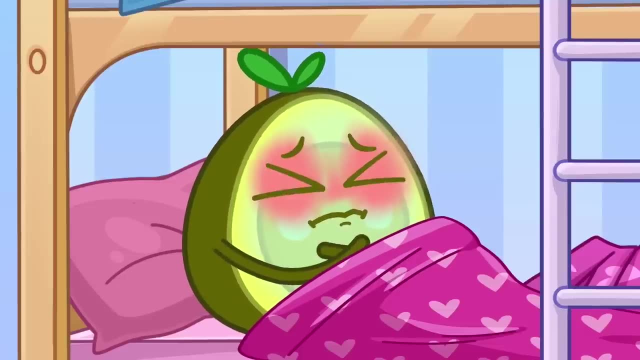 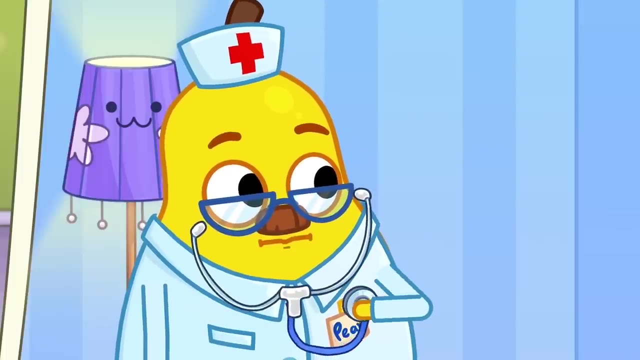 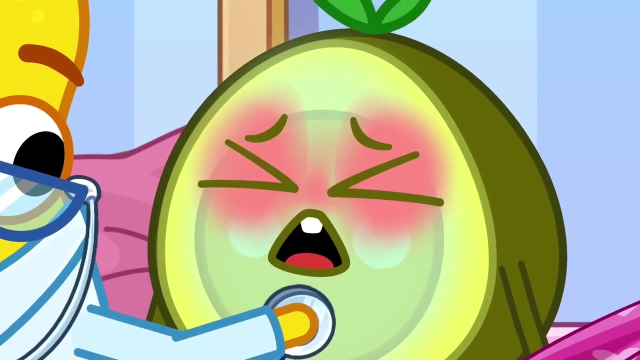 It's Dr Pear. Hey, Hello, Penny. What's the problem? Do you feel sick? No, I'm healthy. Let's play a game: Breathe, Don't breathe, Breathe, Don't breathe. You did great. 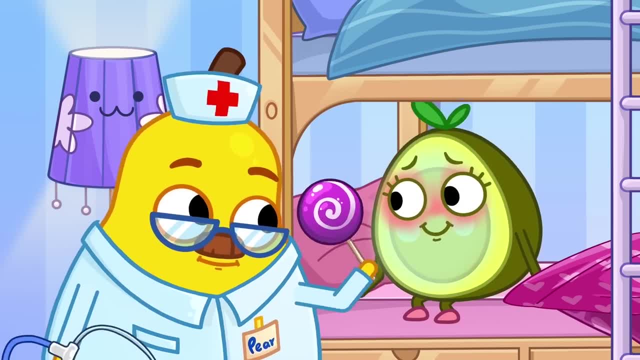 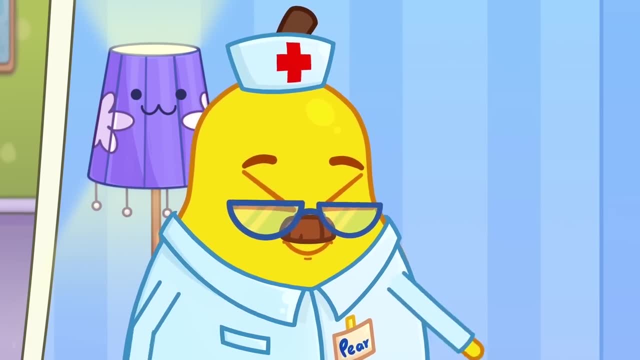 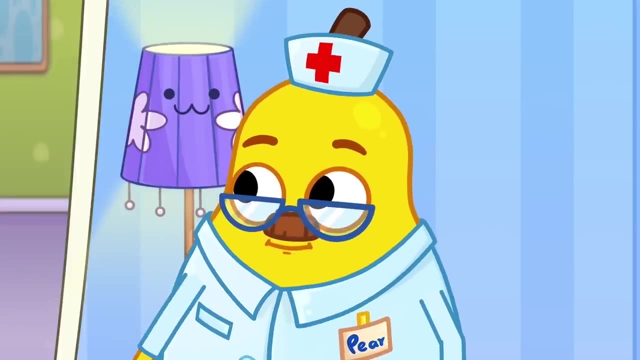 Here's a little gift for you: Wow, A yummy lollipop. This magic lollipop will help you get better. Dr Pear gives Mommy some instructions: Sleep, warm tea and the cold will go away. Thank you, Dr Pear. 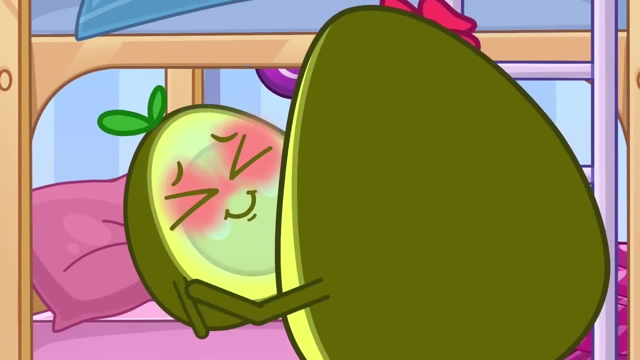 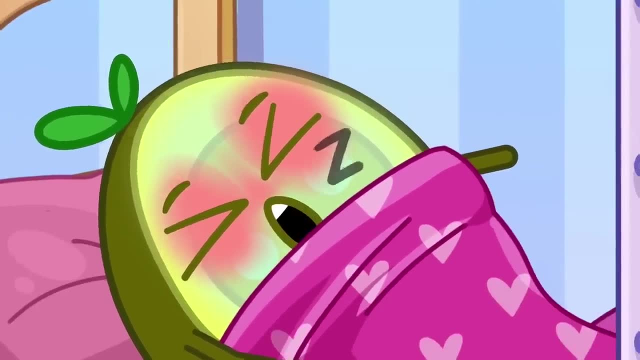 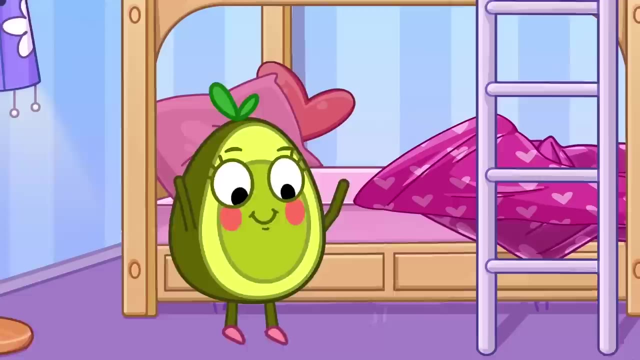 Bye-bye, Bye-bye. We need to listen to the doctor. Oh Oh, It's time for sleep, Penny. I wonder if Penny is feeling better. Wakey-wakey, Penny. Now I'm healthy and ready to play. 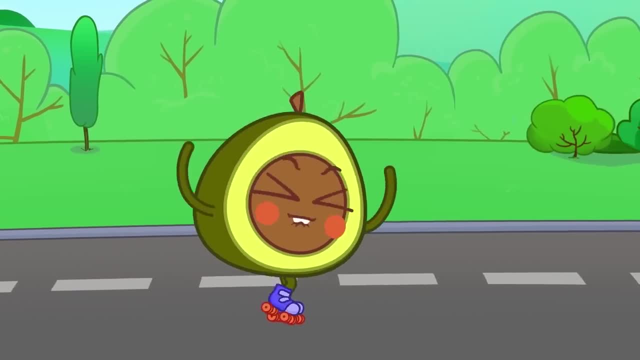 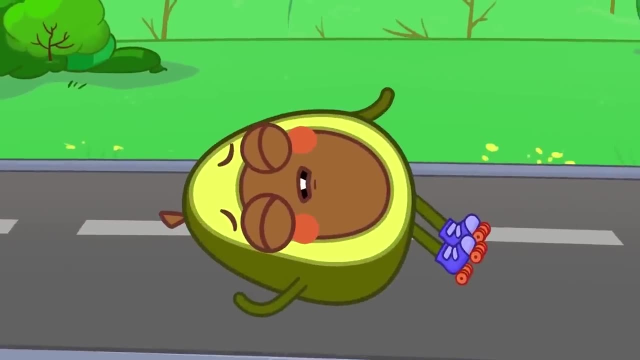 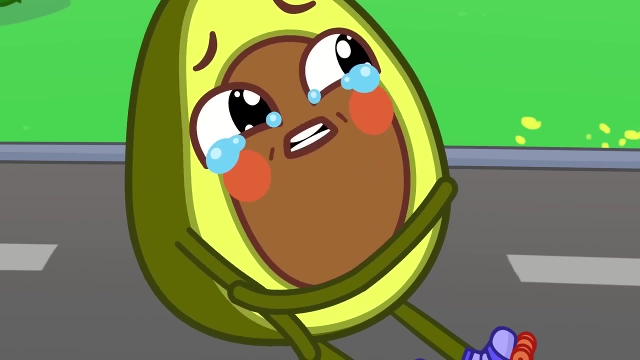 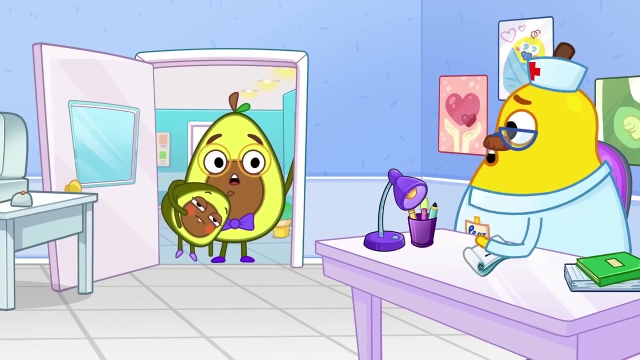 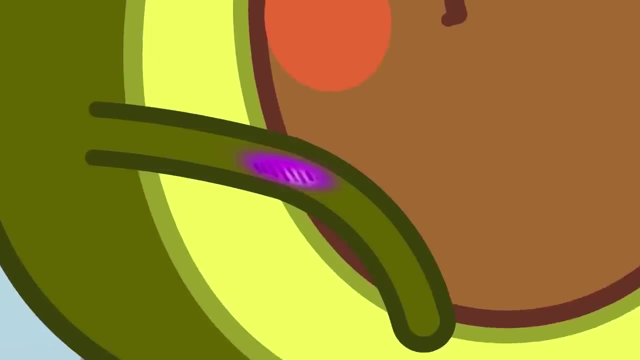 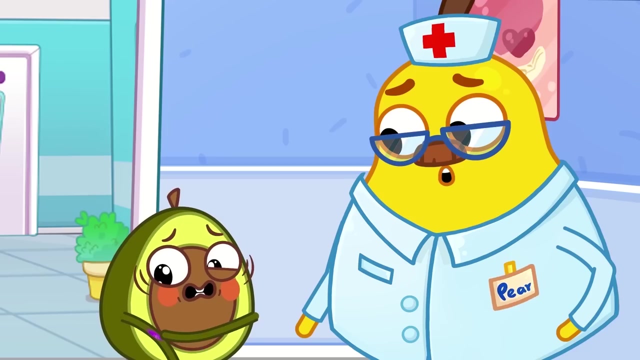 Pit is roller skating. Not too fast, Pit, Careful. Pit has fallen down. My arm hurts. Daddy has taken Pit to the doctor. Show Dr Pear what's wrong. Pit Repeat after me. Dr Pear puts a band-aid on Pit's arm. 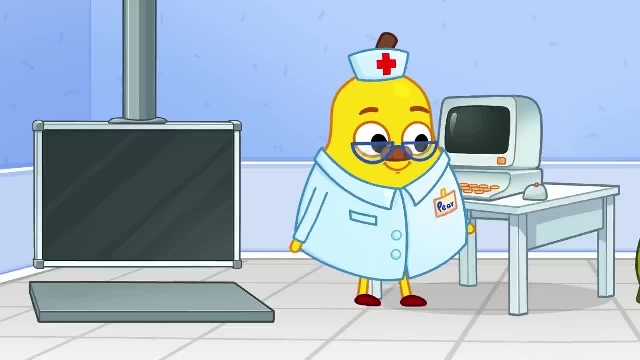 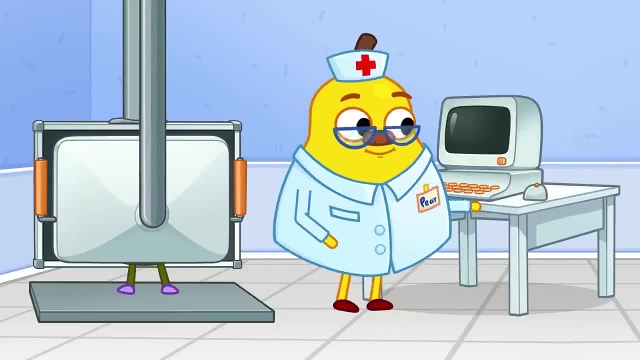 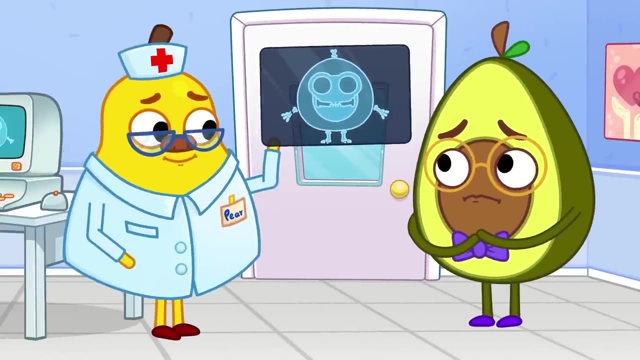 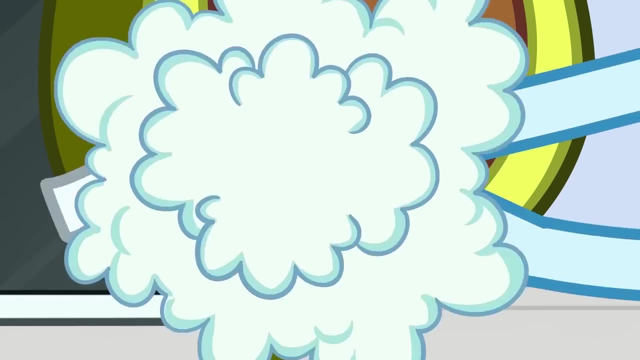 Dr Pear has an idea. He is going to take a special photograph of Pit. This will help Dr Pear find out what's wrong. Don't worry, Daddy Pit has really hurt his arm, But Dr Pear can make it better. 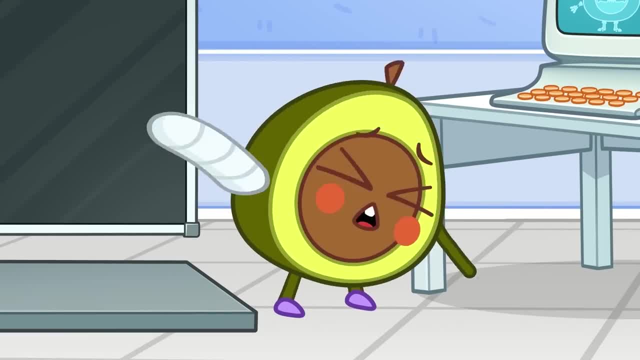 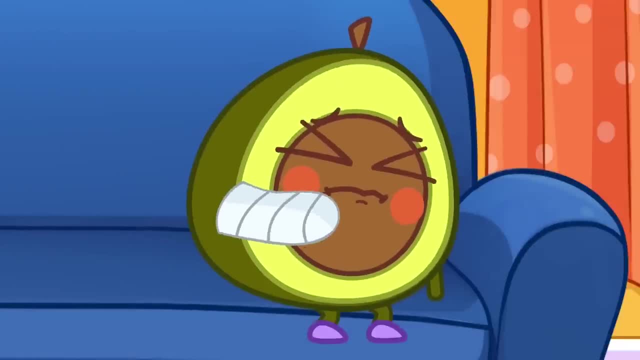 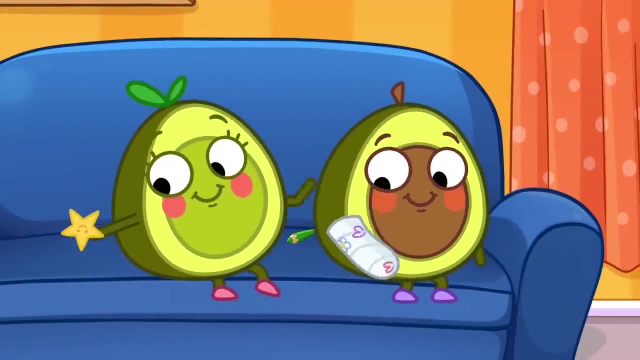 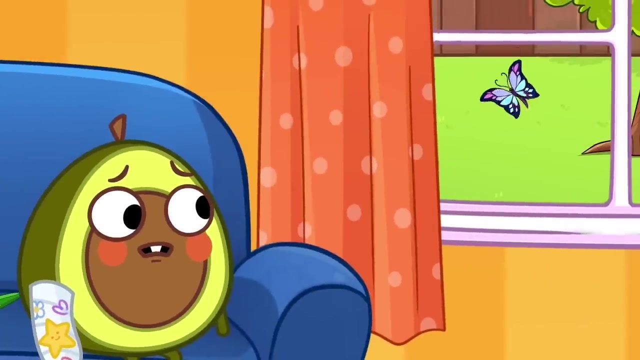 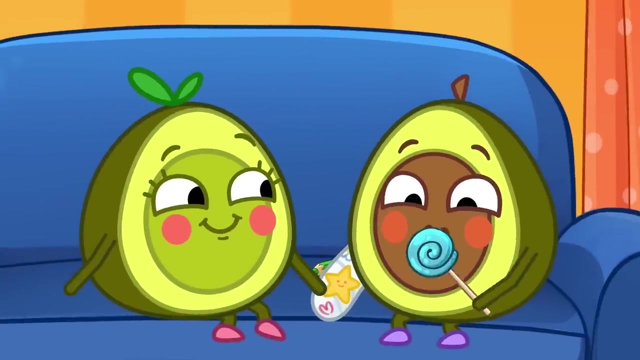 Wow, I'm a superhero. Superhero needs a break. Pit is back home and resting. Penny knows how to make him smile And she has a special star for Pit. Pit wants to go outside. Hope you get well soon. That was very nice. 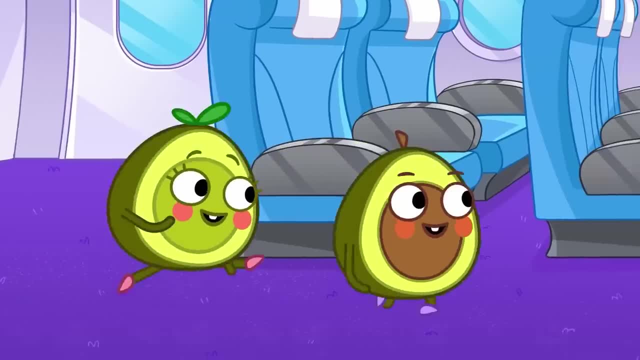 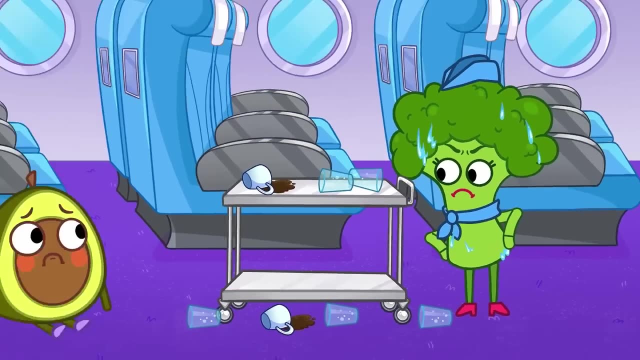 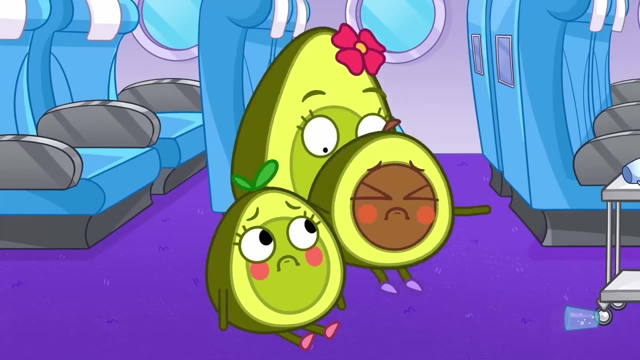 I hope that in the end my mini car will help him heal. Sit tight, penny. It was not easy. Take care of those little sheep. Wait a minute. We can't even go outside Now. I'm sitting in my car. 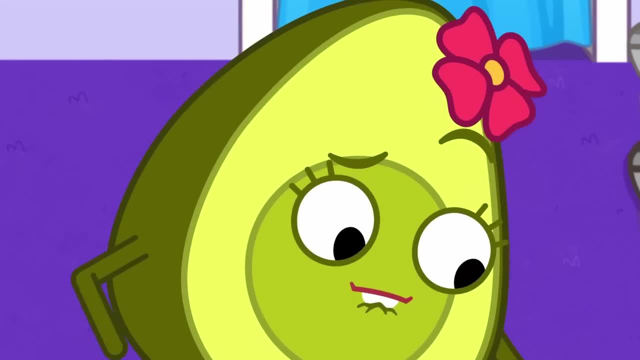 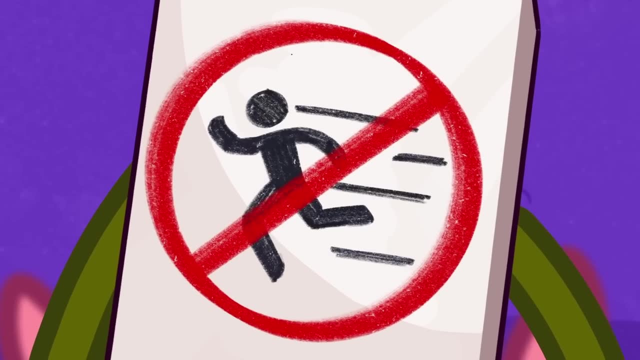 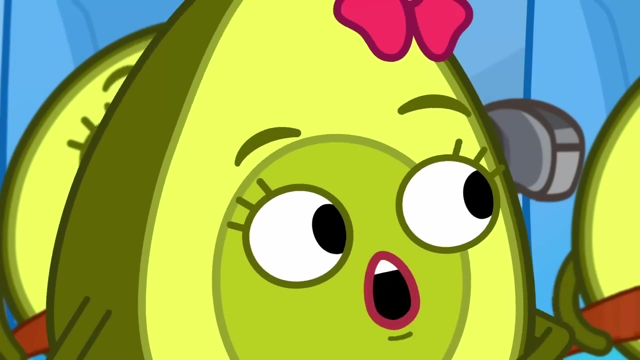 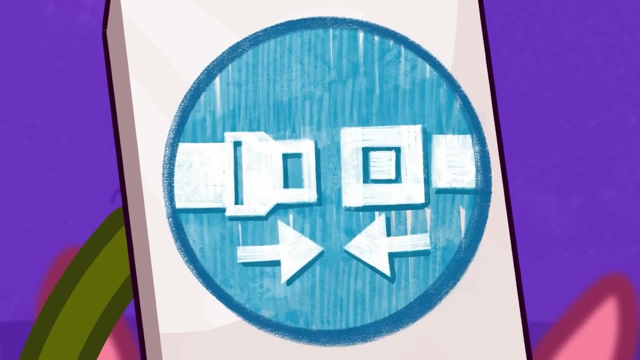 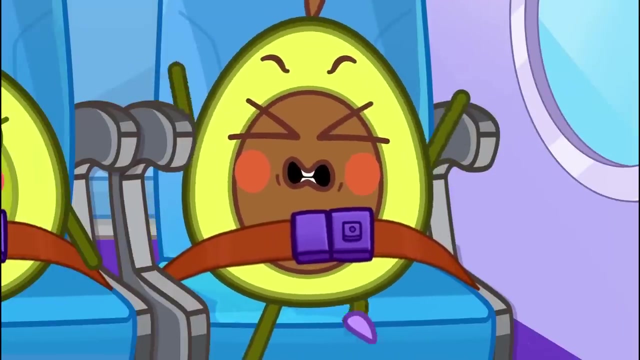 It's already good. Never go outside, Not including yourself, But the bad guys Running can cause accidents. And don't forget your seatbelts. Now you're a save What's wrong? Pit. It's so boring, Stop kicking the seat Pit. 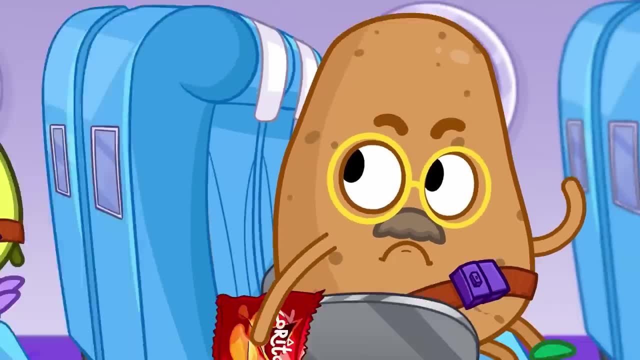 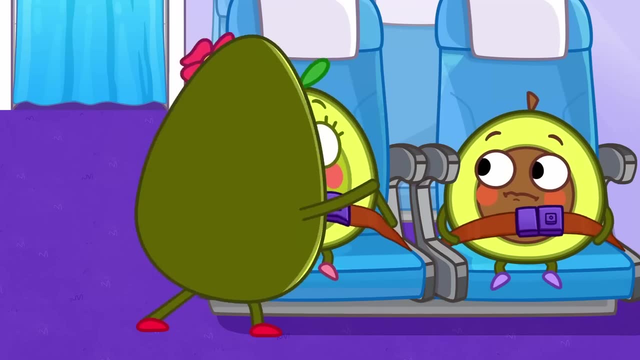 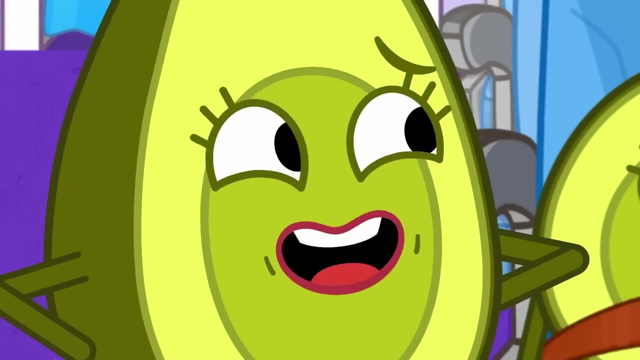 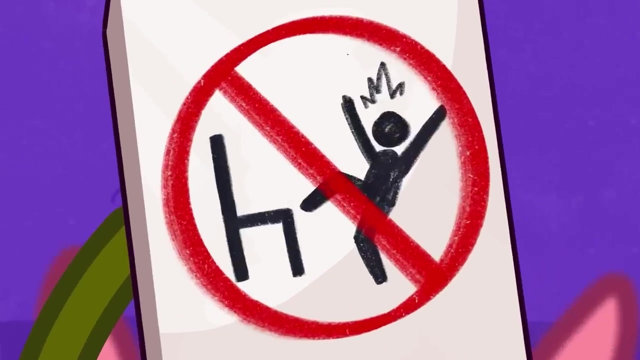 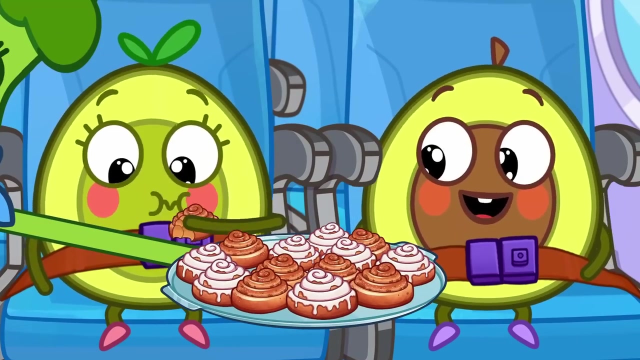 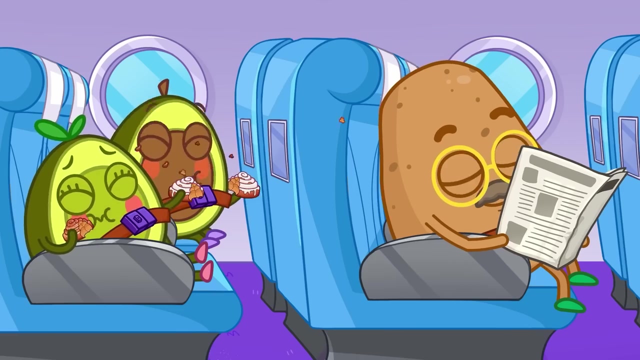 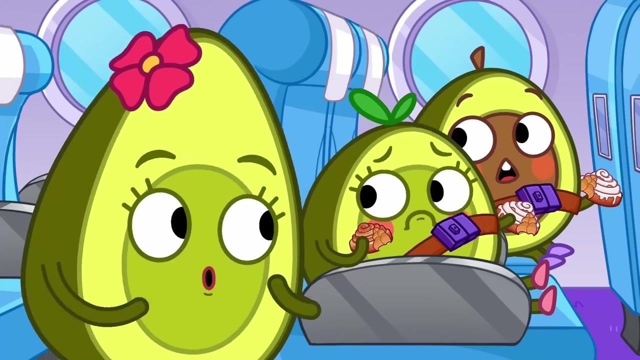 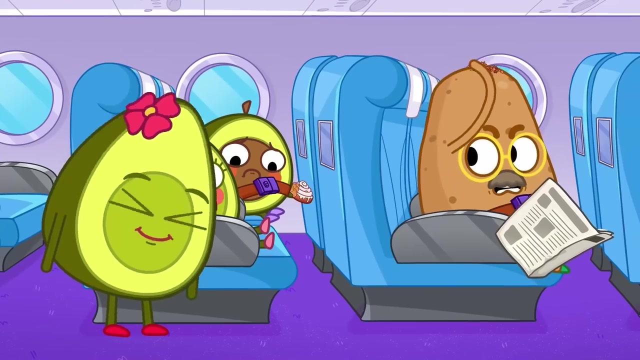 I'm sorry, sir, Kids, you disrupt other people. You should sit up straight. The others can enjoy the flight Snack time. It will lift your spirits. Pit, you're making a mess. Oh Pit, You should be careful while eating. I'm sorry, Don't make a mess on the plane. 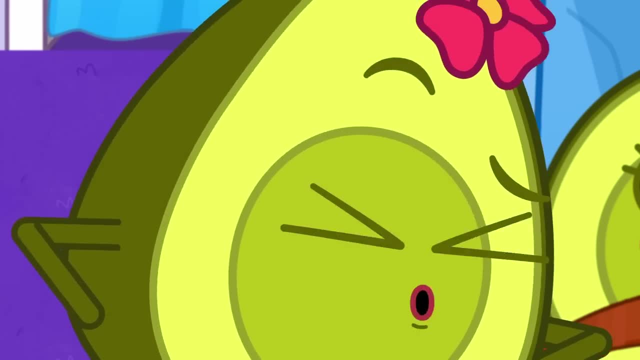 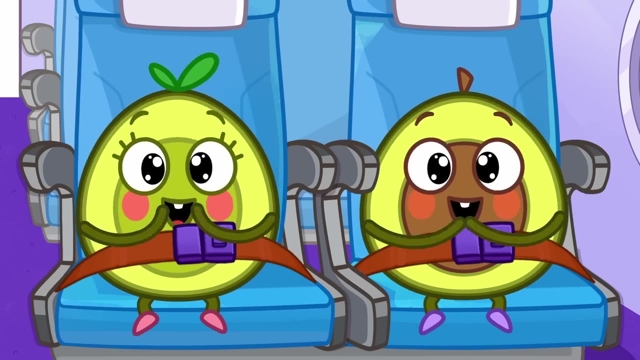 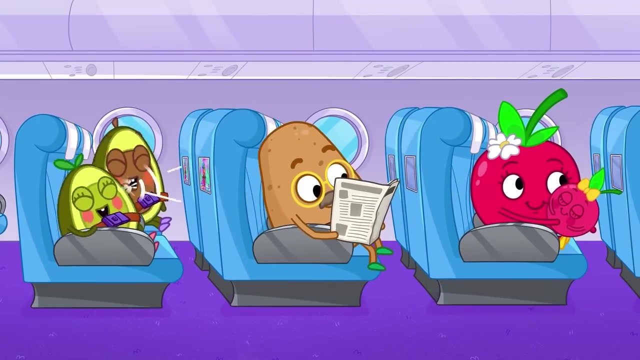 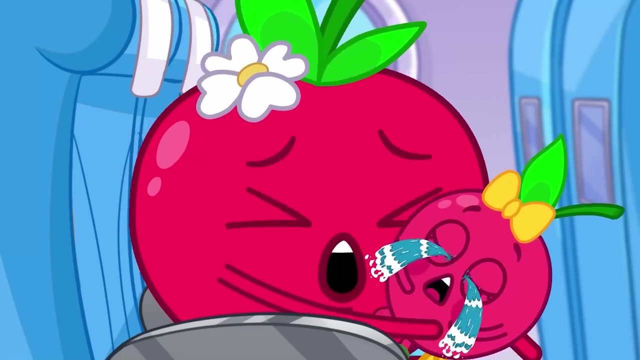 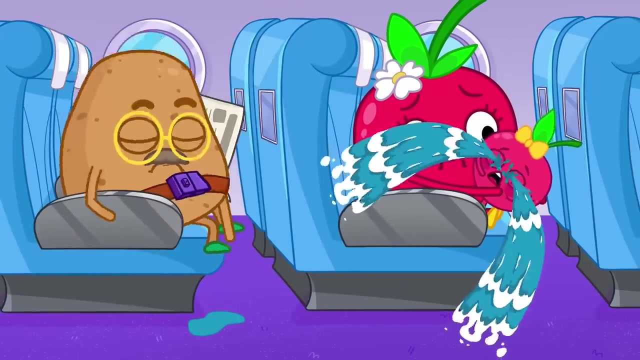 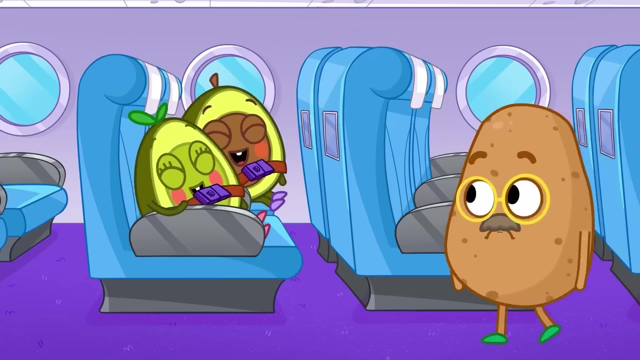 I know what you need. Maybe some TV will help the kids behave. But now Pit and Penny are being too loud. Oh no, The kids have woken you up. Mr Potato is upset. I can't take it anymore. These kids really don't know how to behave. 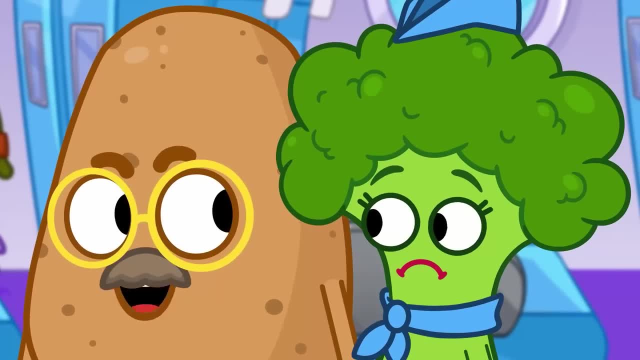 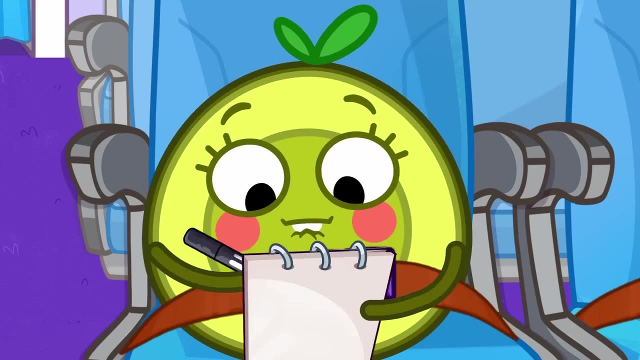 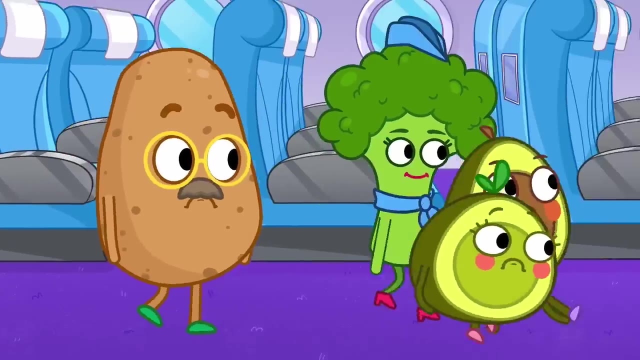 Give me another seat. Oh Shh, We'll be back in a minute Enough talking. Don't talk too loud when you're on a plane. What's wrong guys? Have you ever heard about their private life? Pit and Penny have something to say. We're sorry. 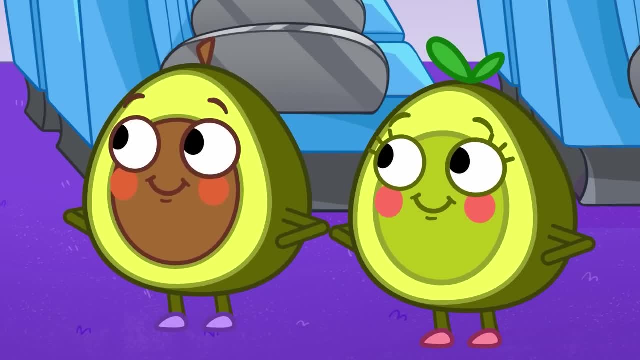 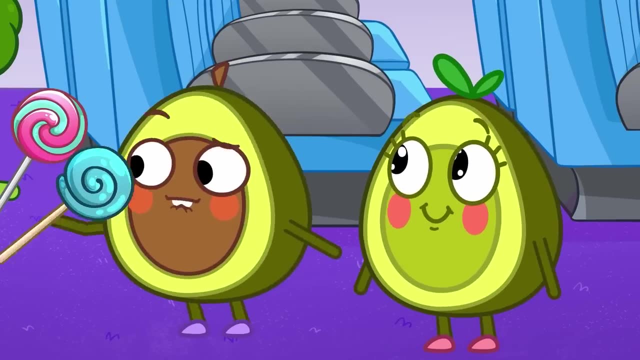 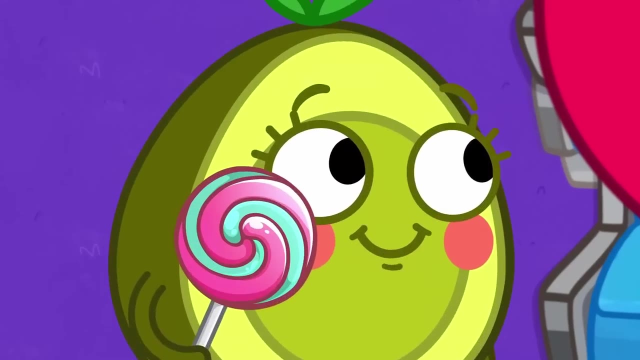 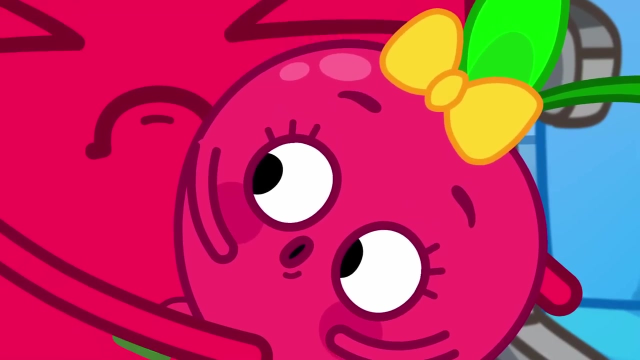 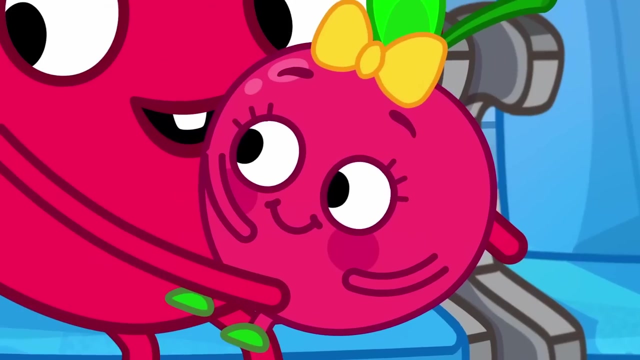 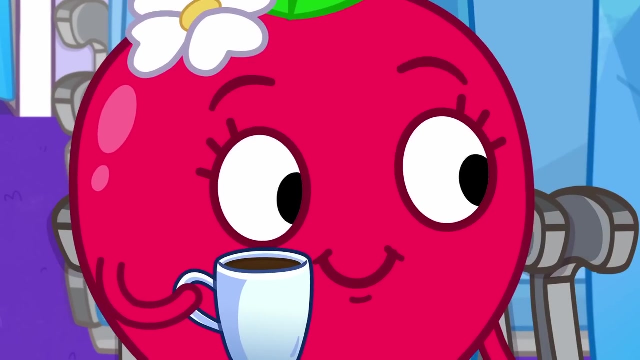 Now we know the rules. We're so sorry. Here's two lollipops for being well-behaved. What was that? I was so scared. We started the party. What? Let's go home. Whatever's on the table should be in the room. you, the baby, stopped crying. now everyone's happy. your children are so well behaved. 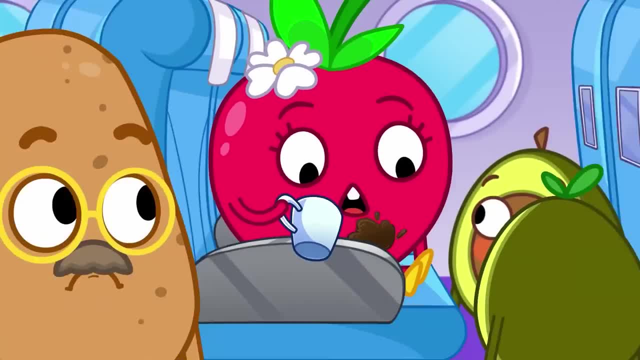 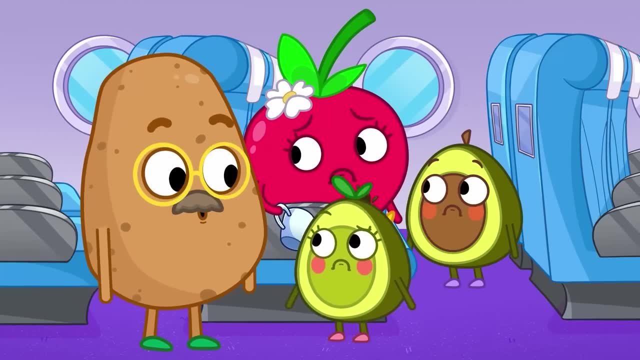 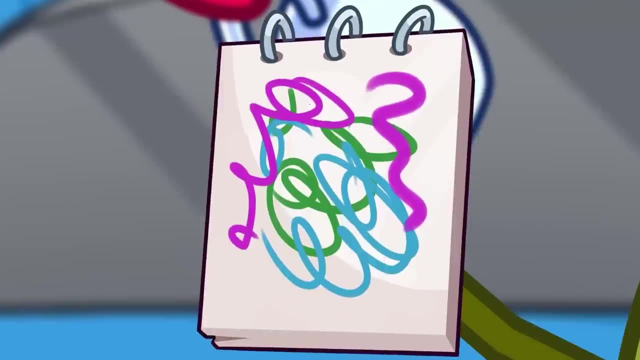 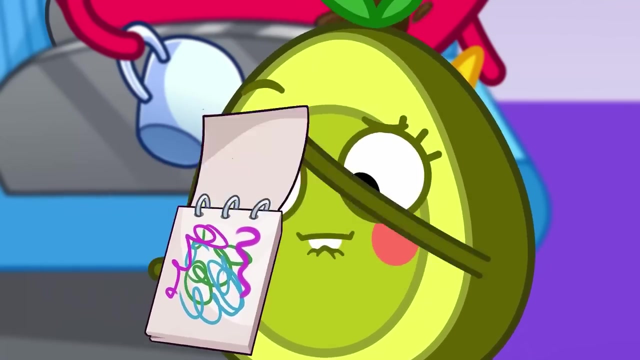 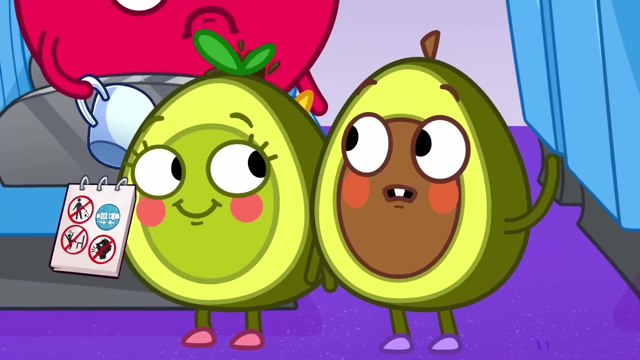 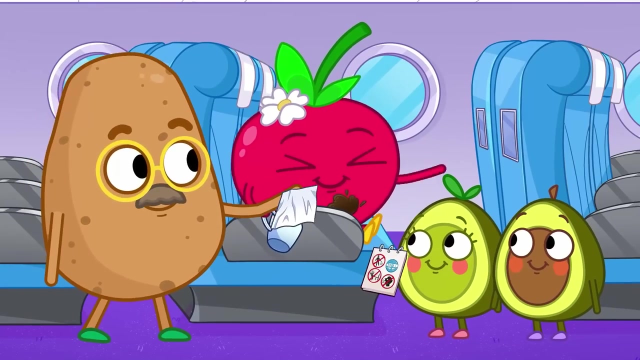 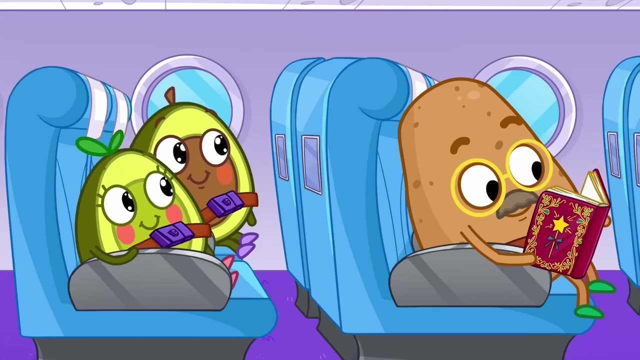 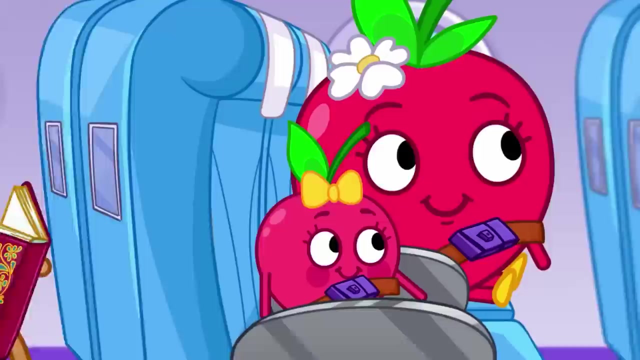 you should be careful, sir. everyone must follow the rules, always be respectful of others. you should know the airplane rules, sir. thank you, kids, and sorry ma'am. i think it's time for a story. once upon a time, far, far away, baby cherry is ready for her nap, and so are pit and penny. 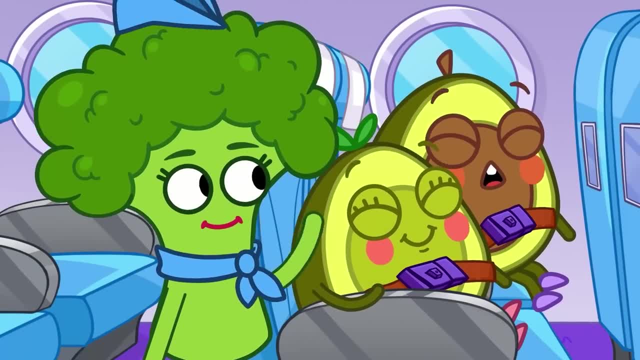 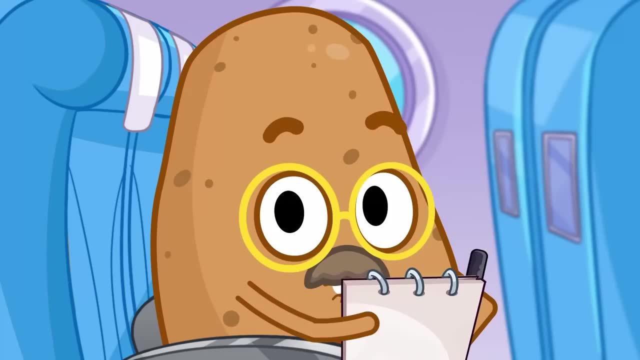 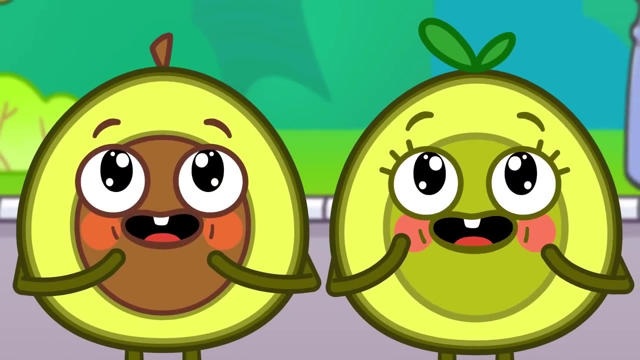 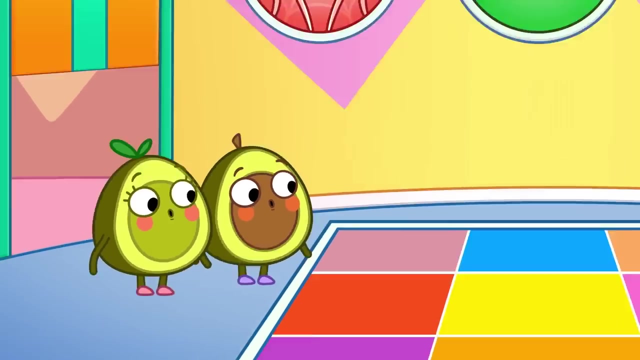 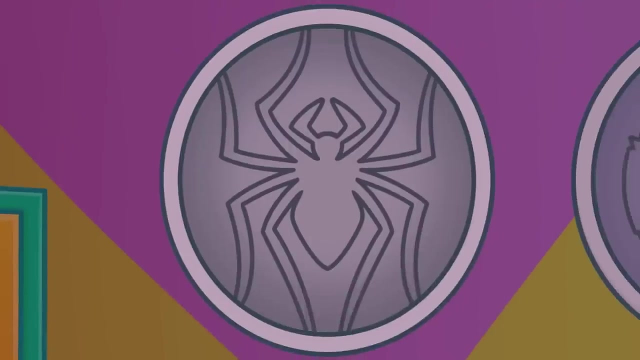 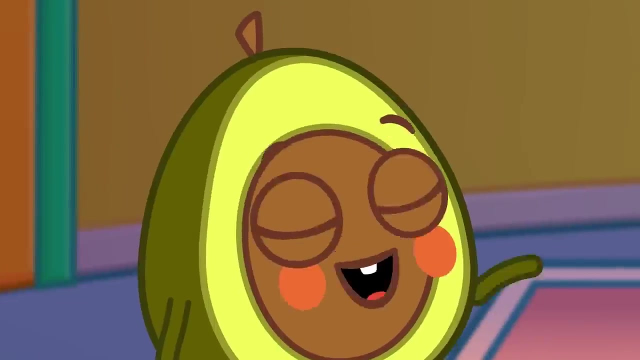 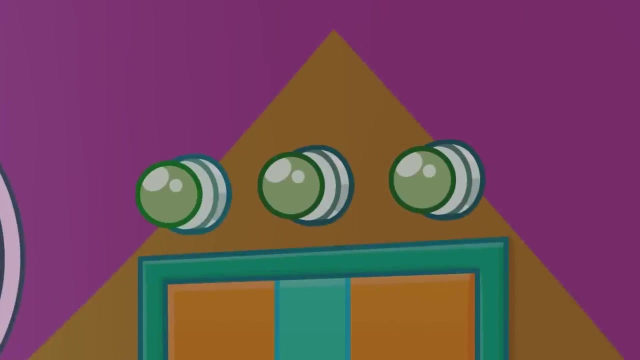 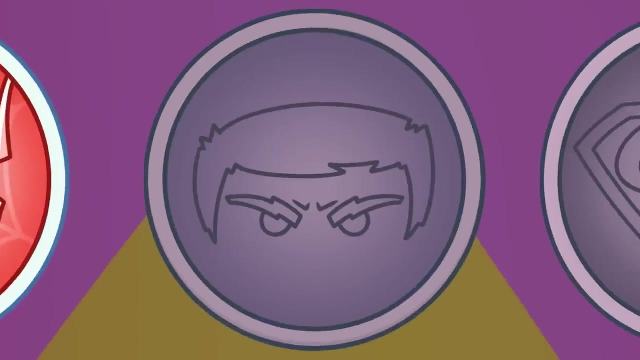 enjoy your flight everybody. look, kids, a quest room, go and check it out. this is the first challenge. oh, but what do they have to do? we need to guess the color. but which one? i know that's right. the spider guy symbol is red. what color is the bulk? this one needs green. 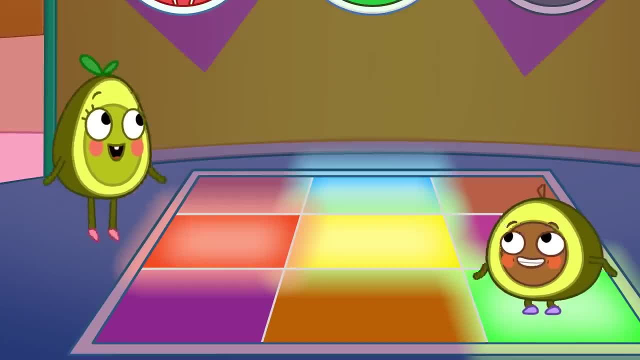 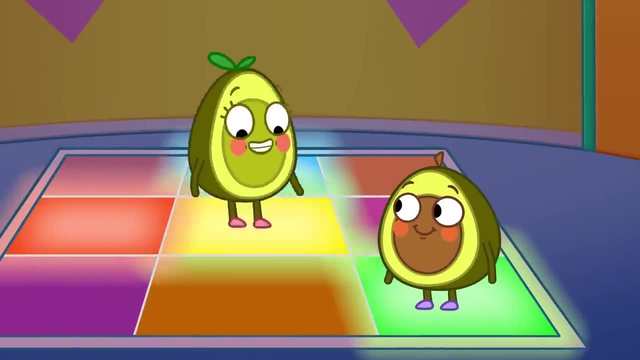 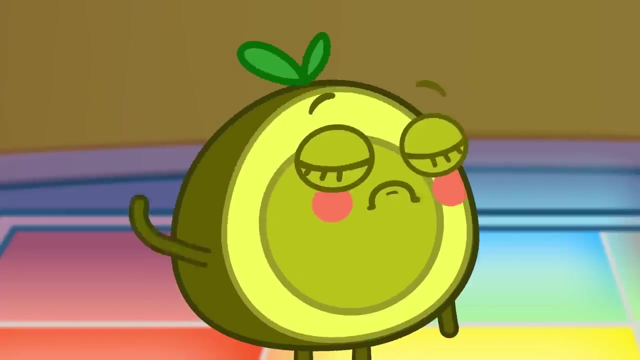 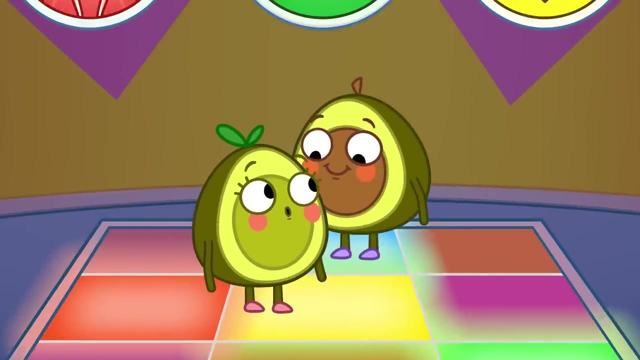 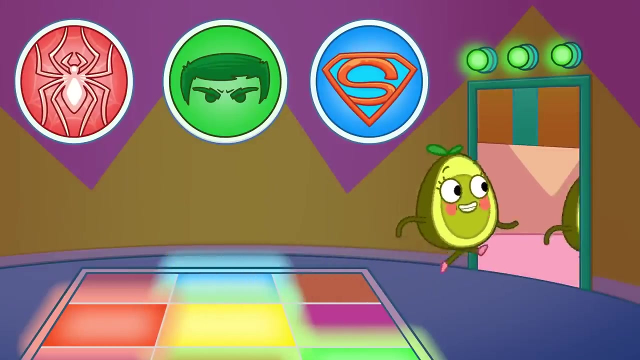 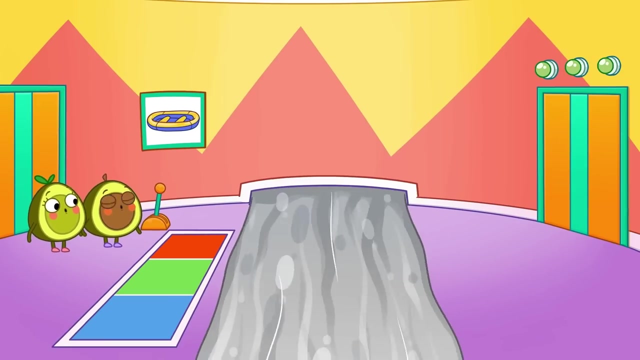 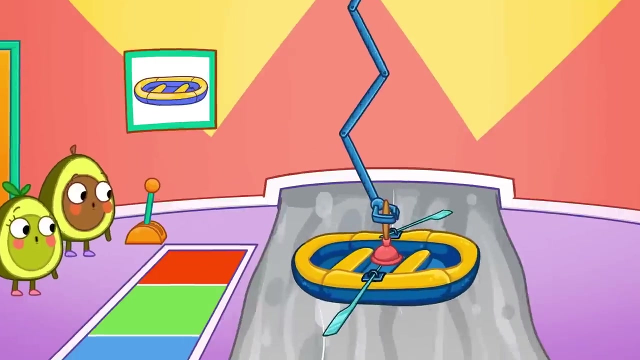 that's right. the bulk is green. it needs yellow. wrong, super guy's suit is not yellow. try again, kids. no, we need the blue color, is that right? it is. oh now, what must they do? what is this for? oh, they need to choose the color of water. 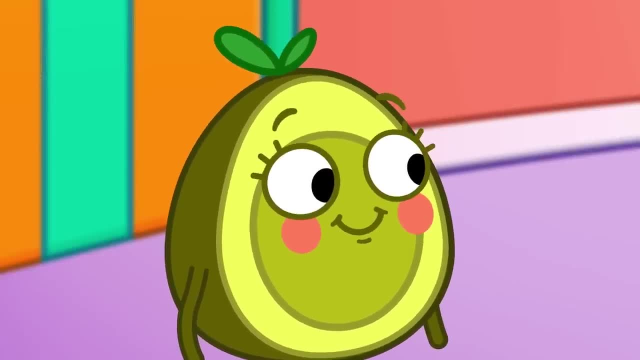 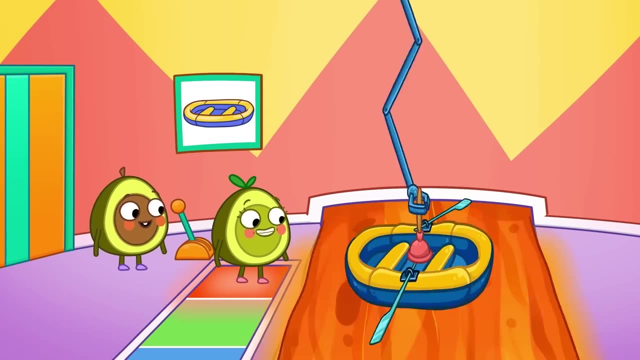 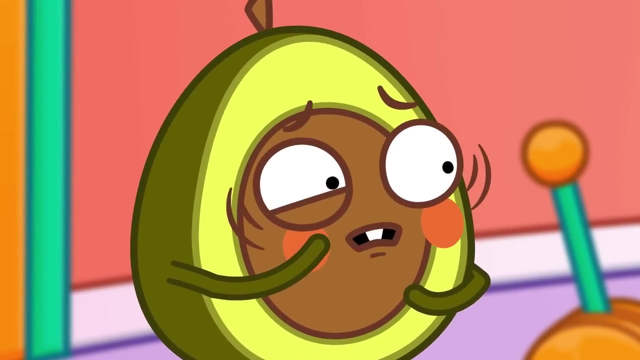 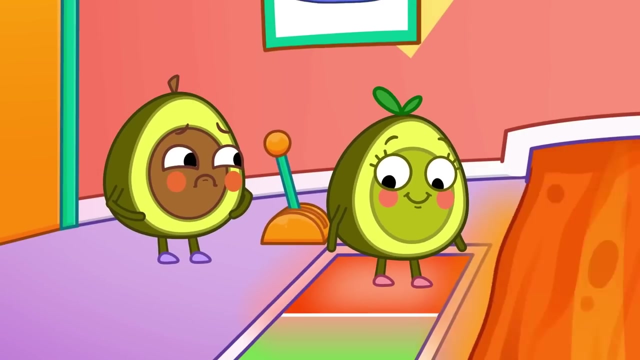 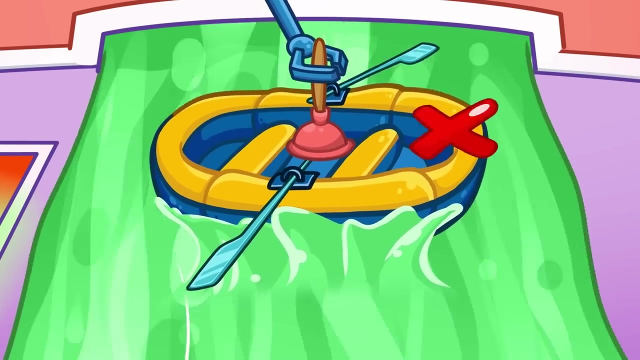 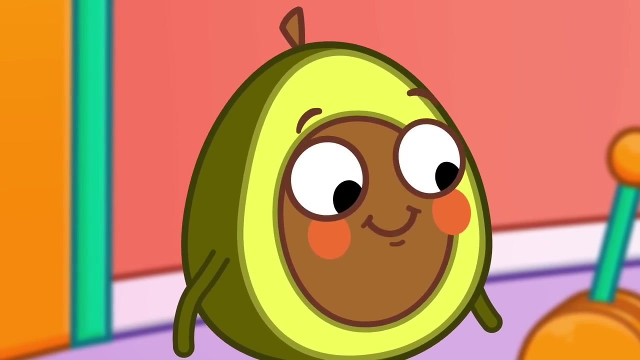 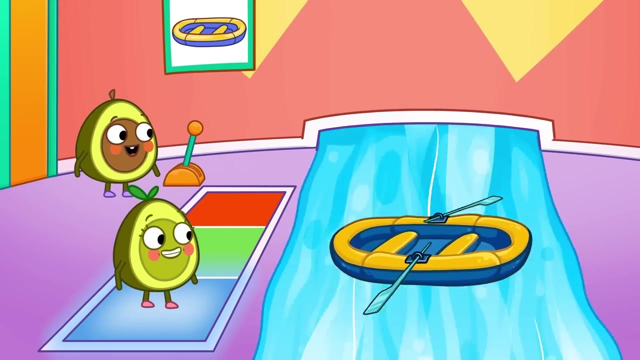 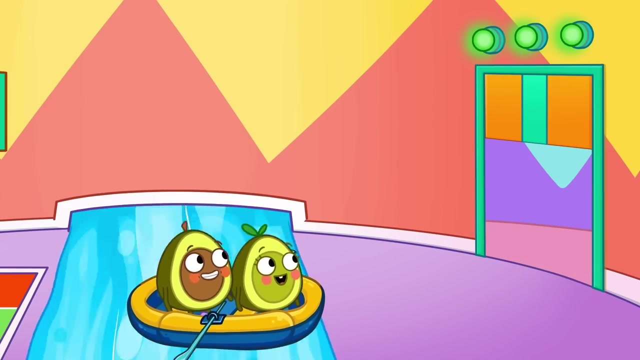 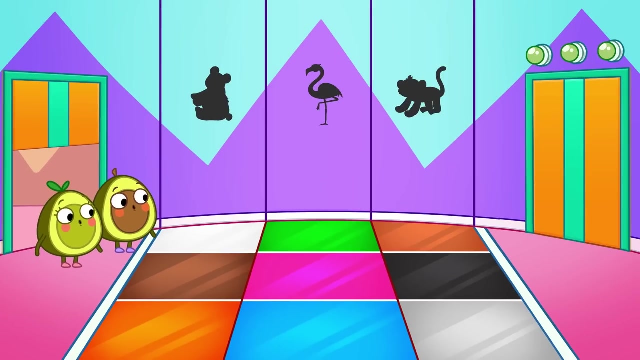 we have to choose the correct color. maybe red, that's too hot. oh, it's lava. we need to pick another color. oh, maybe green, that's too slimy. i know we need blue. oh, that's right. water is blue and boats float on water. oh, now color the animals: it's a bear. 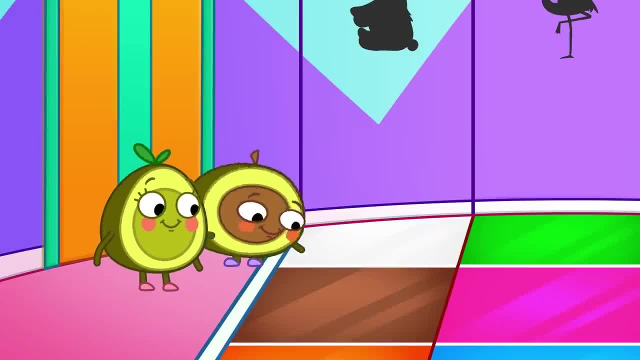 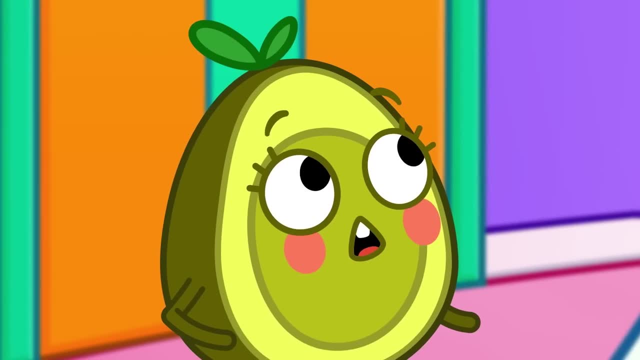 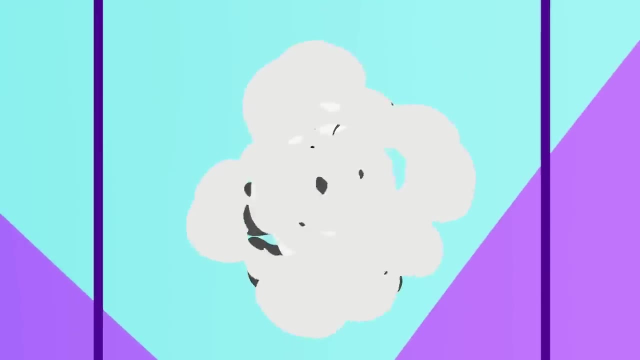 what color is it? now? color the animals? it's a bear. what color is it? hmm? hmm. what color is it? Hmm, it's not a brown bear. I know the color. Why? white? White for the panda. What's next? Pink for the flamingo. 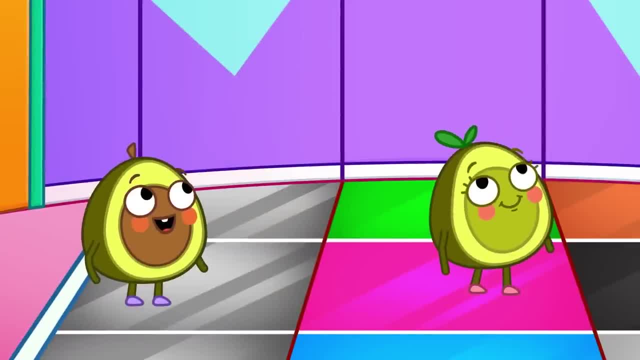 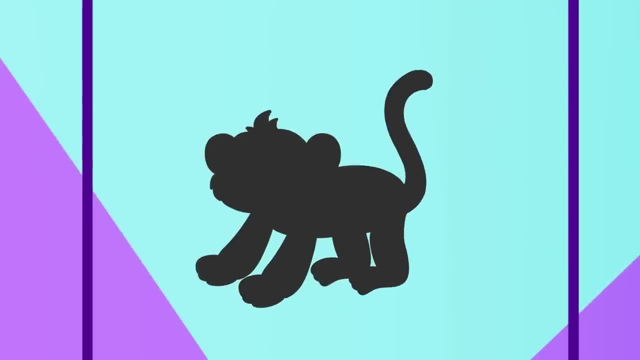 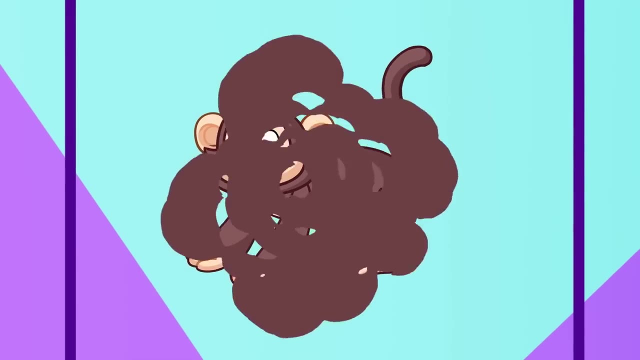 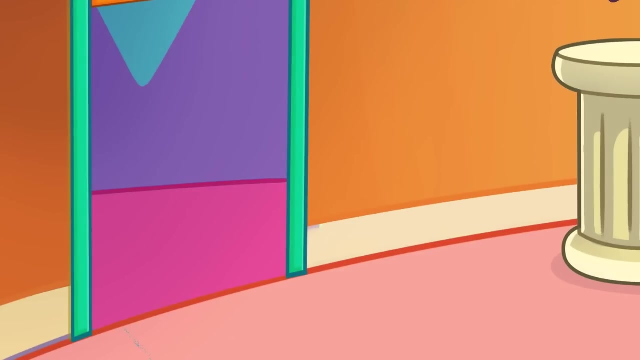 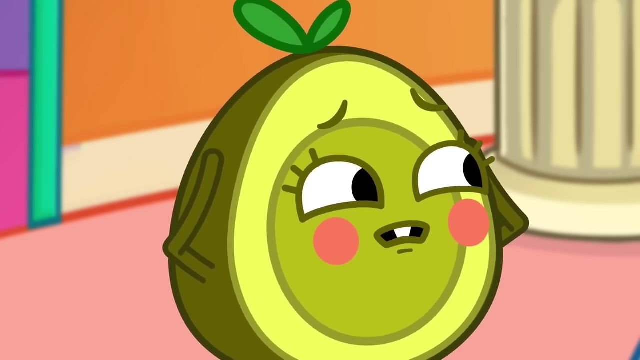 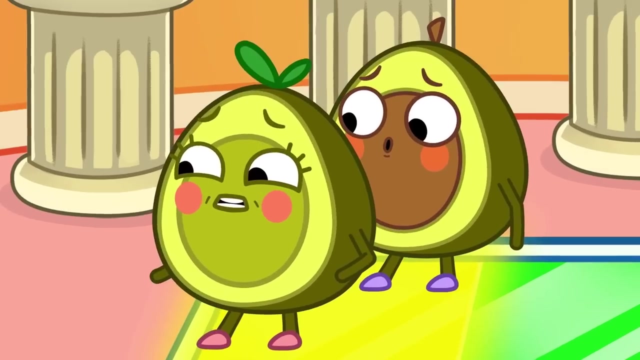 Yes, Flamingos are pink. Brown for the monkey, This monkey is brown, An angry monkey Run. Maybe they'll be safe in here. What, What, What do we do now? Here comes the monkey: A yellow banana. 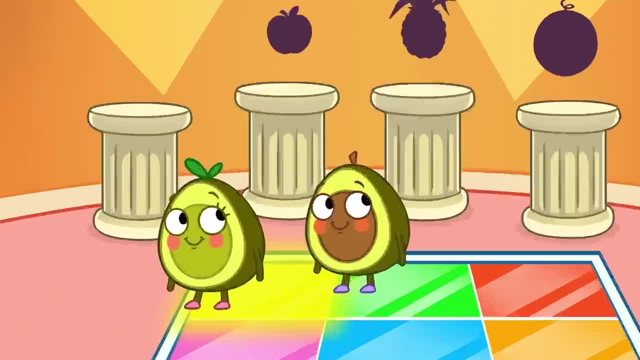 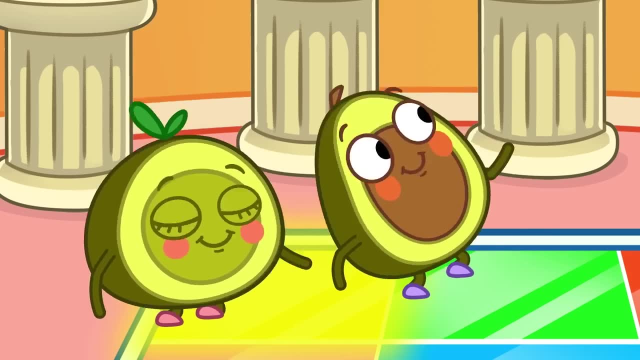 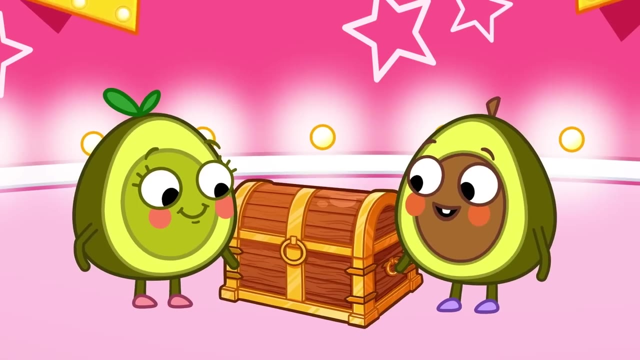 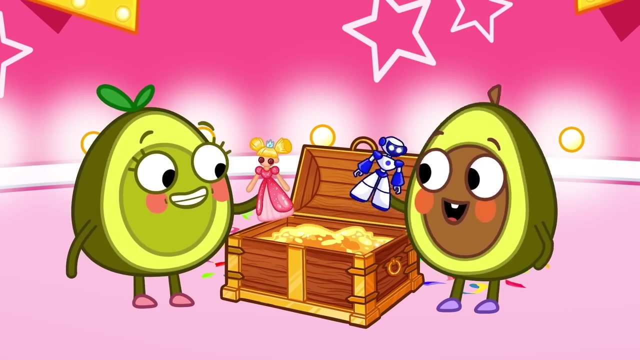 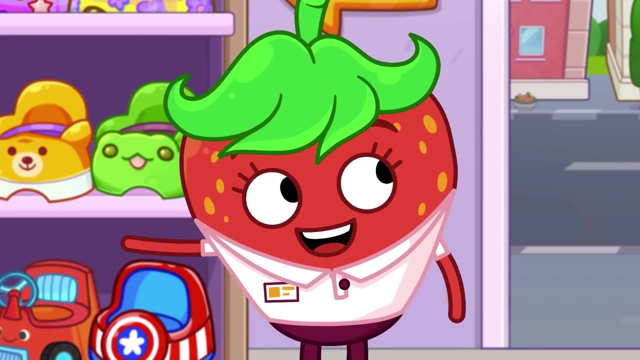 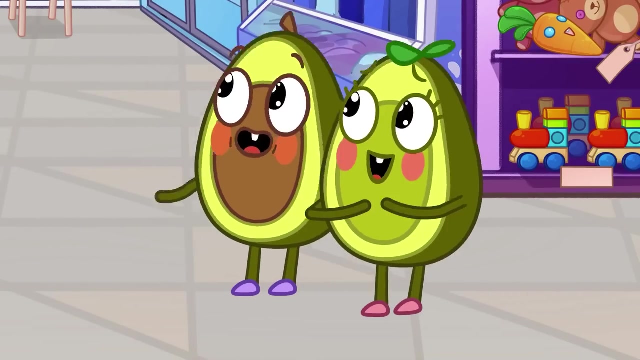 Monkeys love bananas. It was a hungry monkey. A hungry monkey. You finished the quest, Pit and Penny, And here is our reward. Yay, What a great job. kids. It's time to find Baby a potty. Just follow the sign. 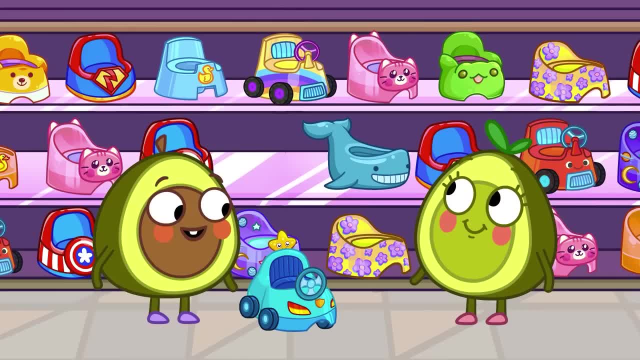 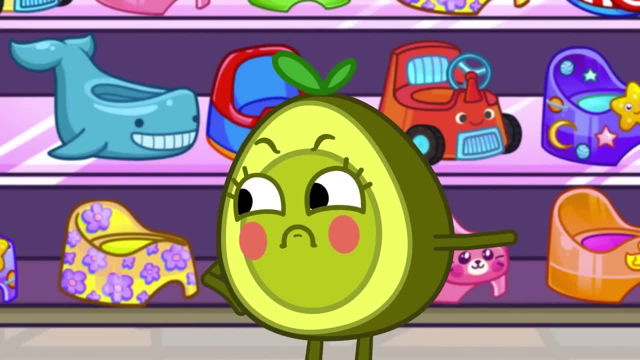 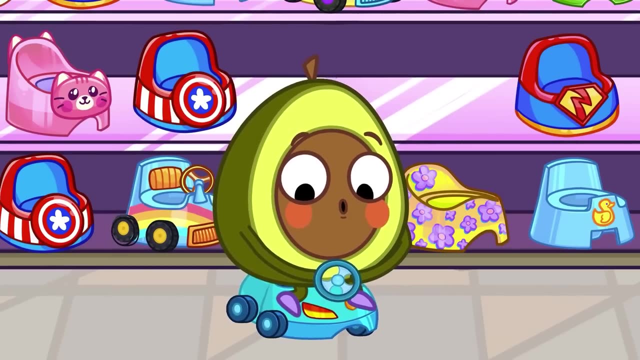 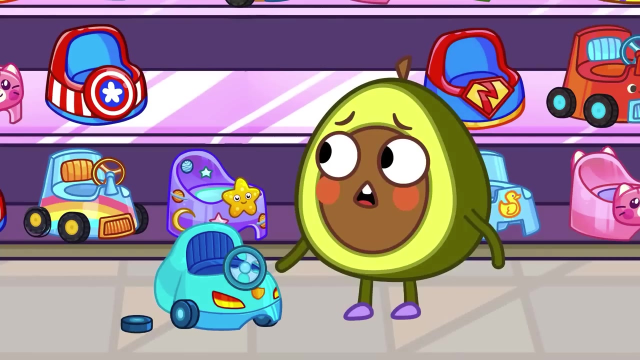 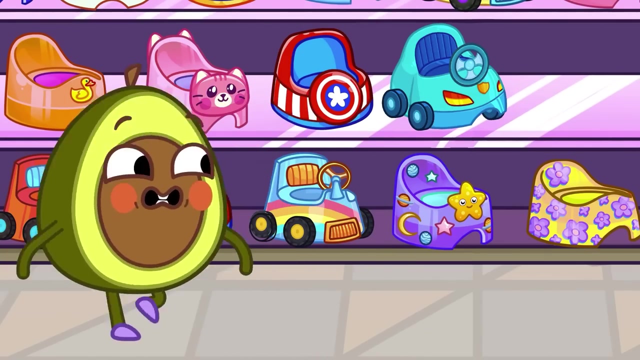 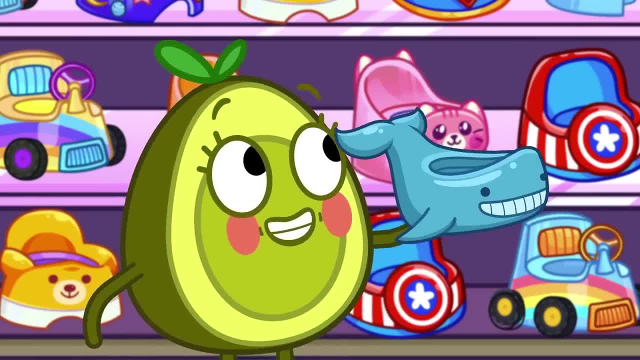 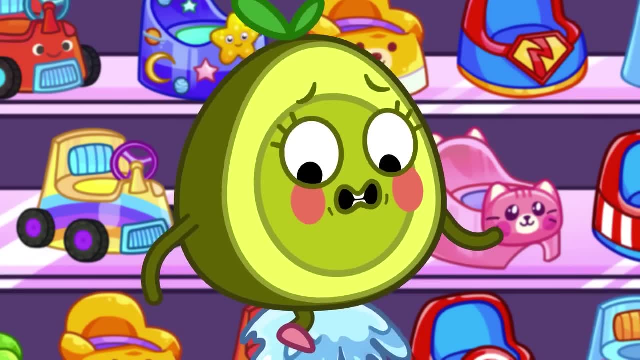 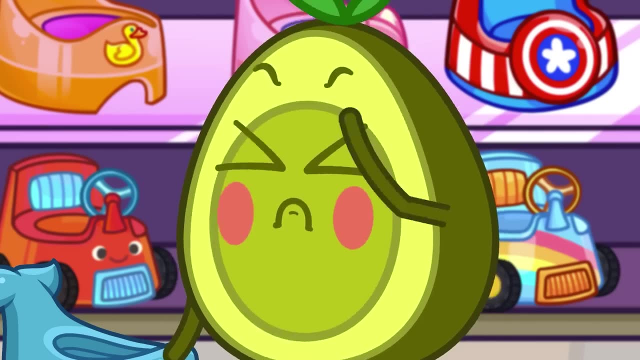 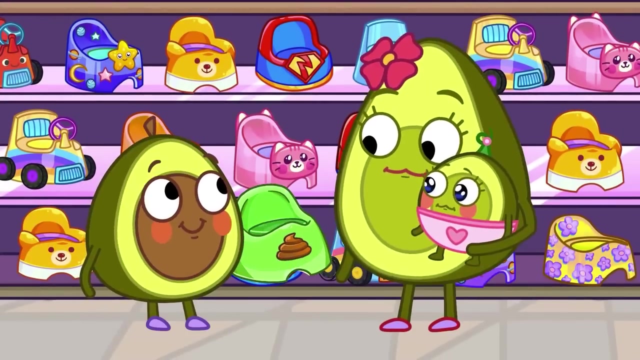 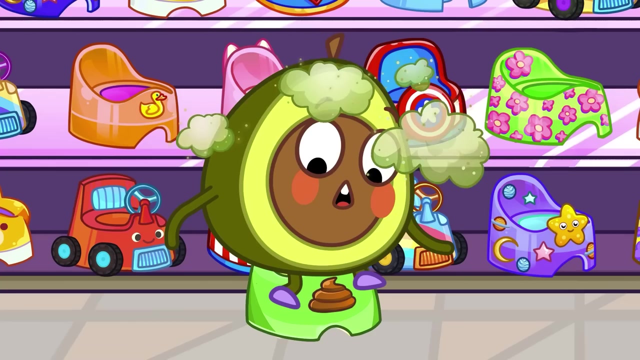 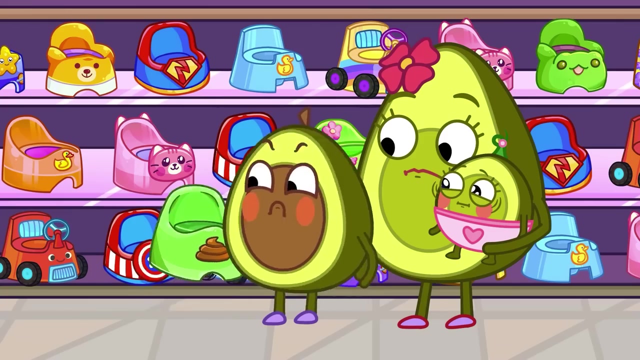 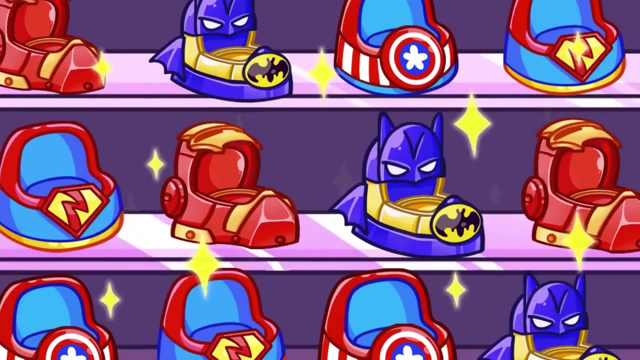 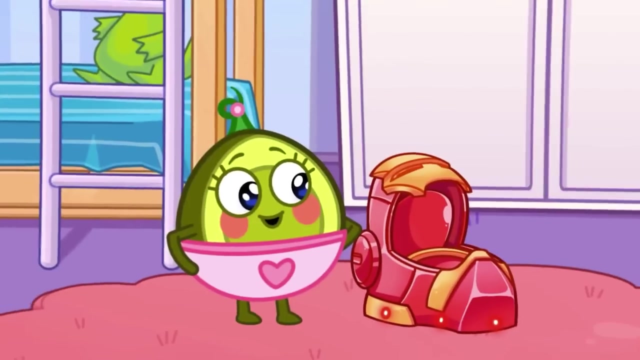 What, What. Maybe Baby would like a whale potty. What's wrong, Benny? That potty is too wet. What about this potty? No, it's too stinky. Look at all the superhero potties. Ooh, it's iron baby. 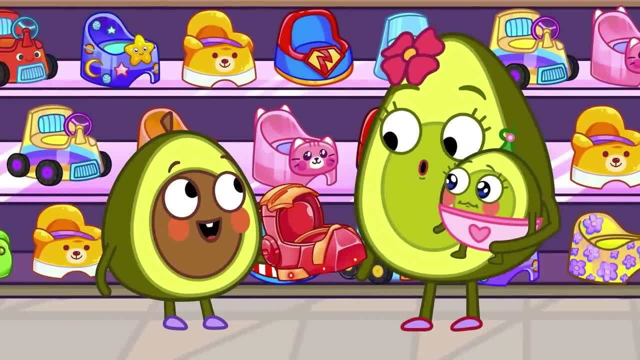 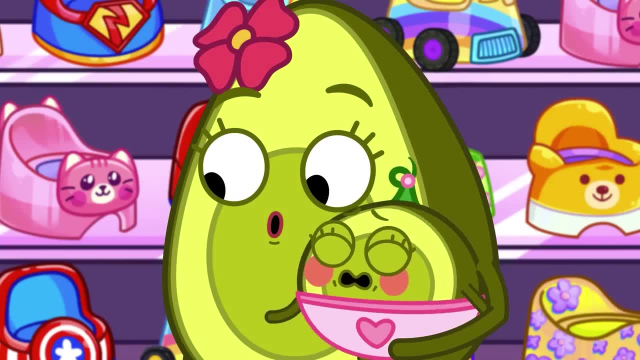 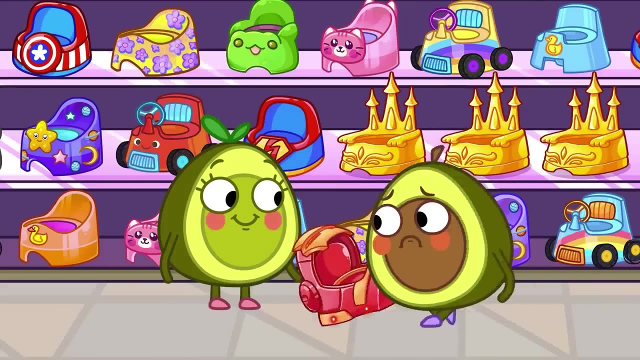 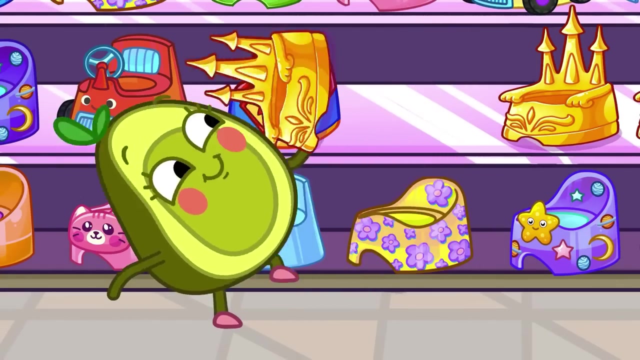 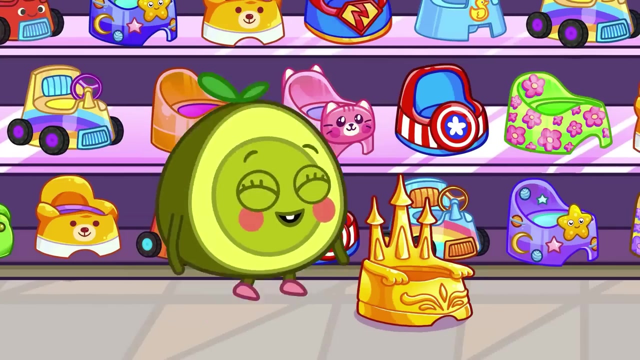 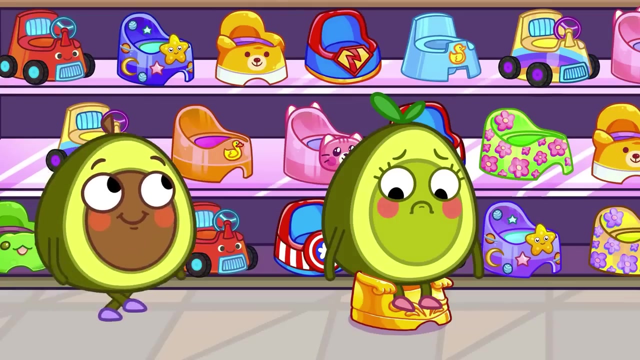 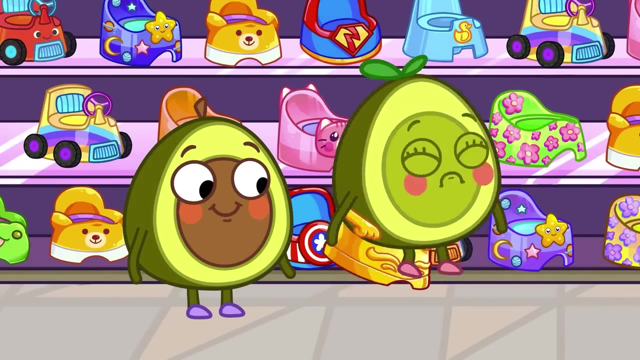 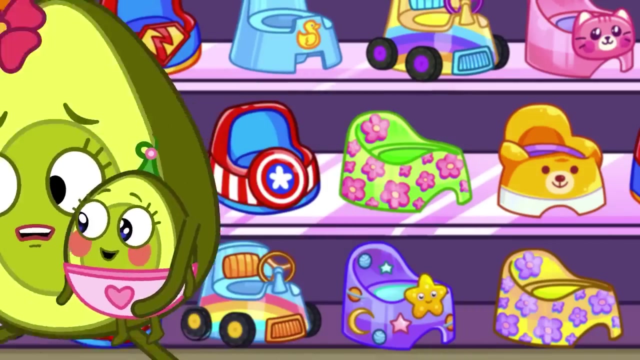 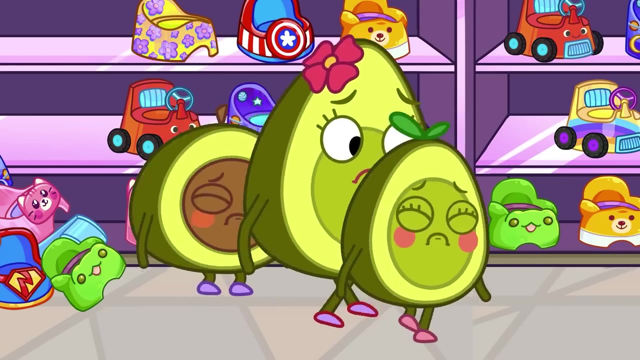 Yay, yay. This potty is too loud and had too many lights. This one looks like a golden castle. Penny's stuck. Can Pit help pull it off? Oops, look at that mess. The store owner wants the family to leave. 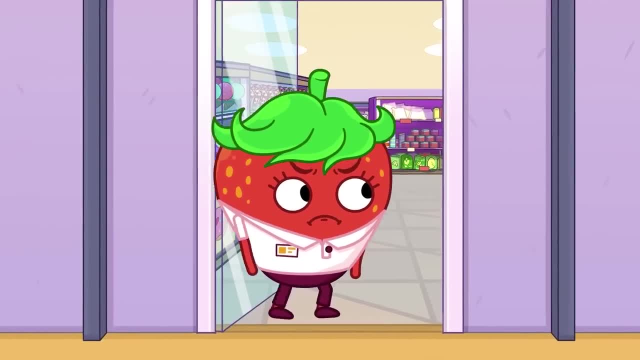 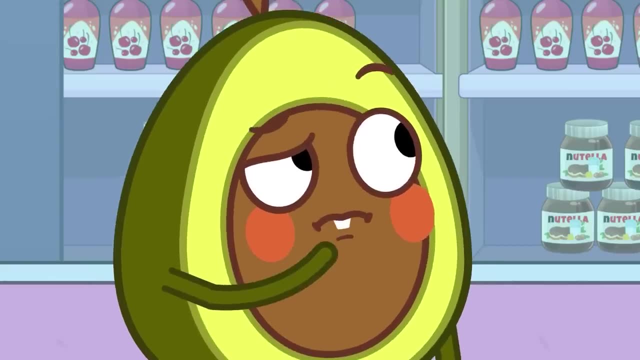 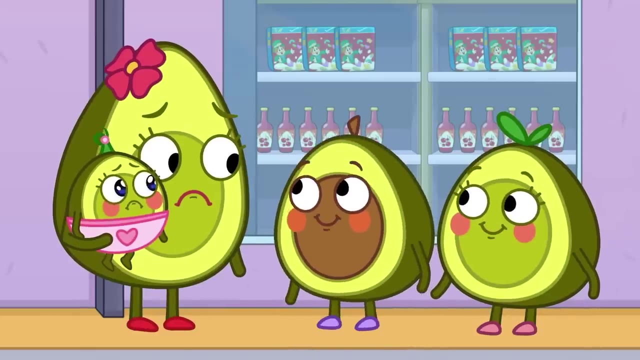 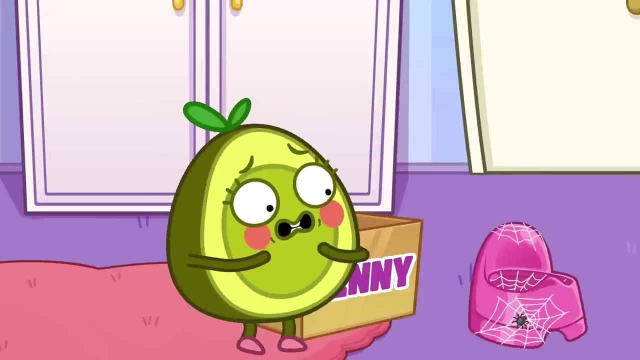 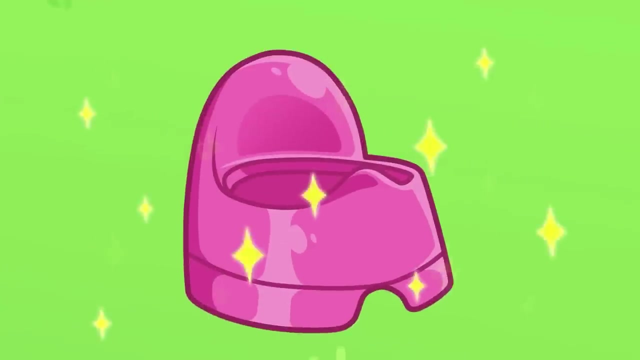 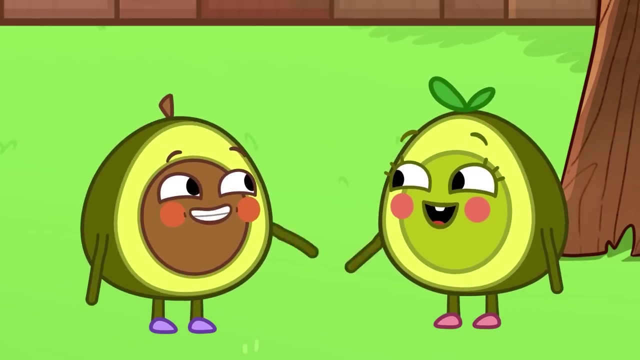 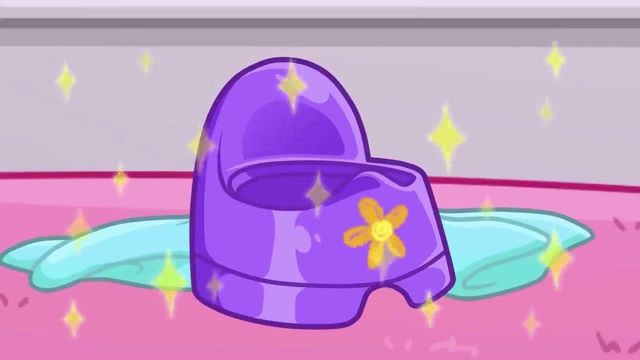 Awww, Pit knows what to do. We will make our own pot. You can start with Penny's old potty. Wow, Clean off the spiders first, Paint it purple and add a flower. Let's see what Mommy and Baby think. Try it, Baby. 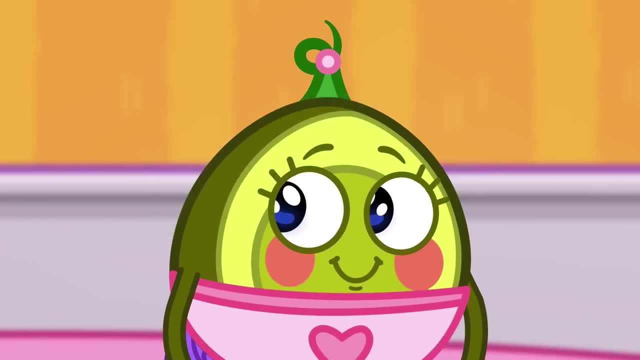 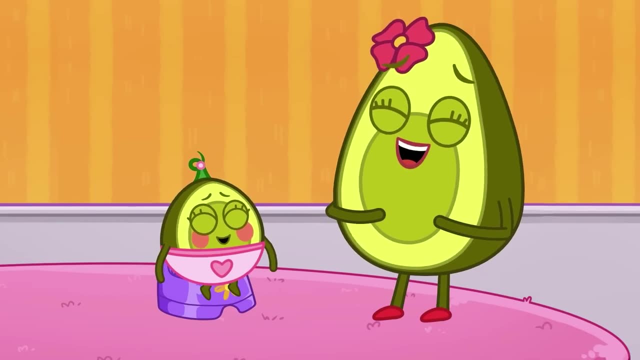 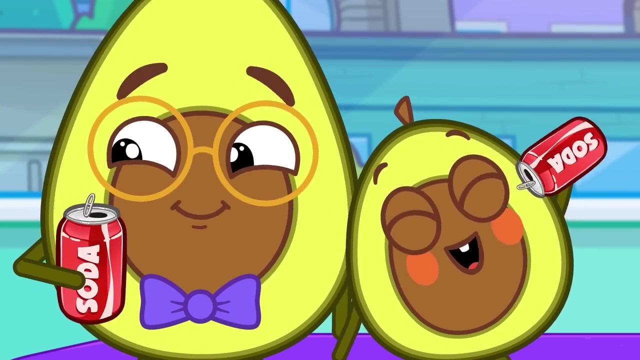 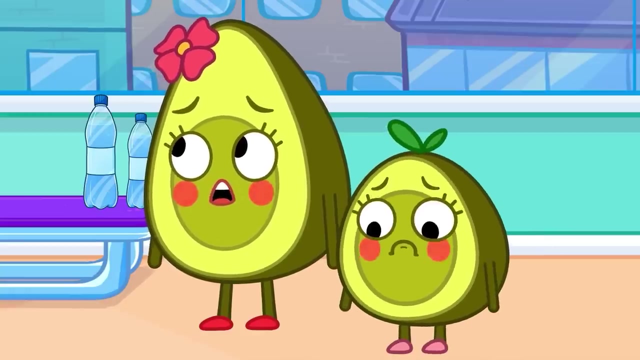 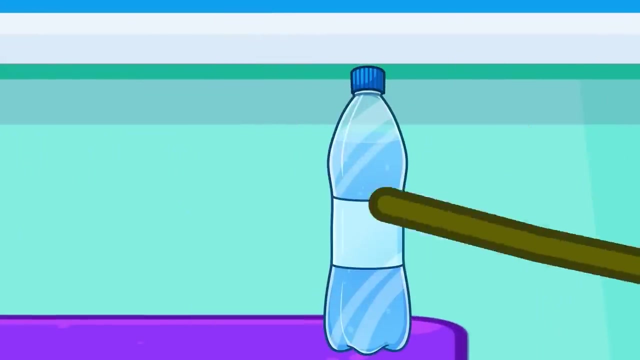 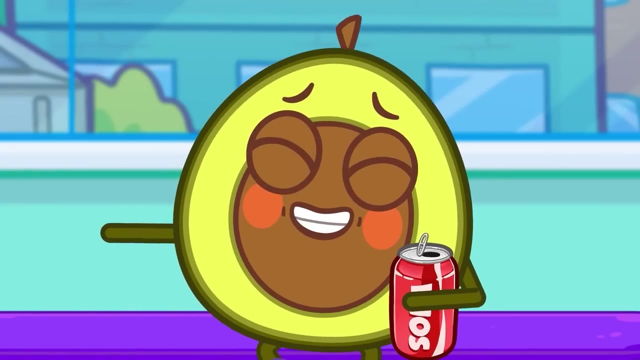 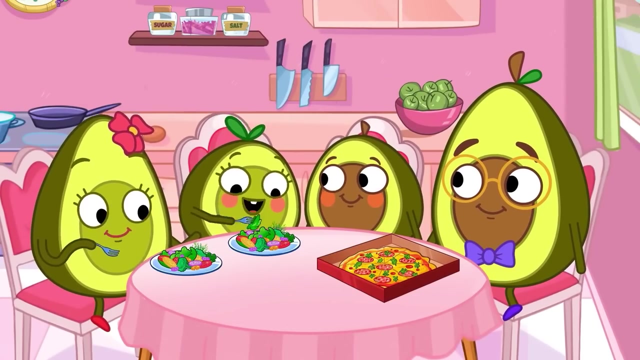 Baby loves it. Well done kids. Penny and Mommy are exercising, While Pit and Daddy drink soda. Now Penny and Mommy are thirsty, But they don't want soda, They want water. Too much soda can hurt your tummy, Even yours, Pit. The girls are eating salad. 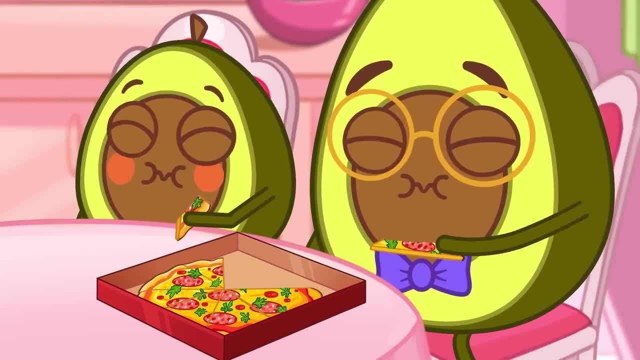 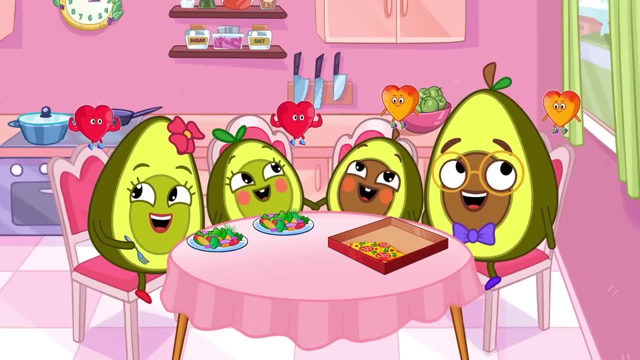 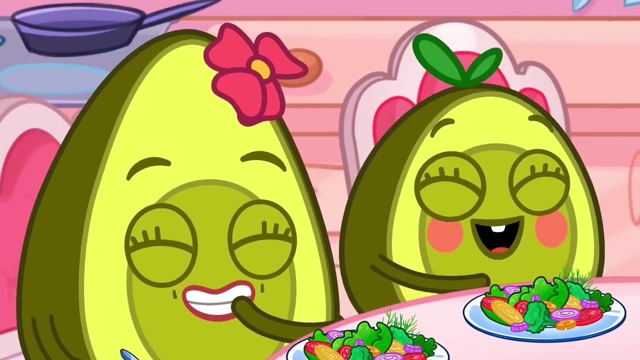 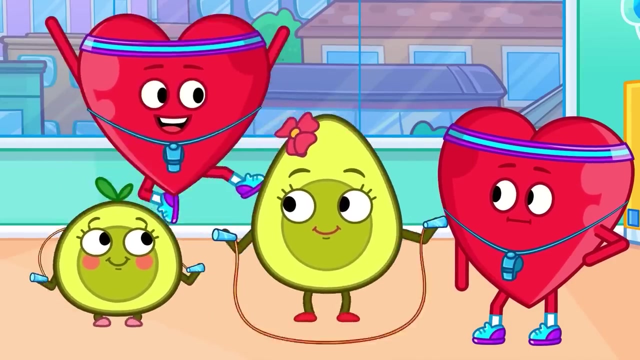 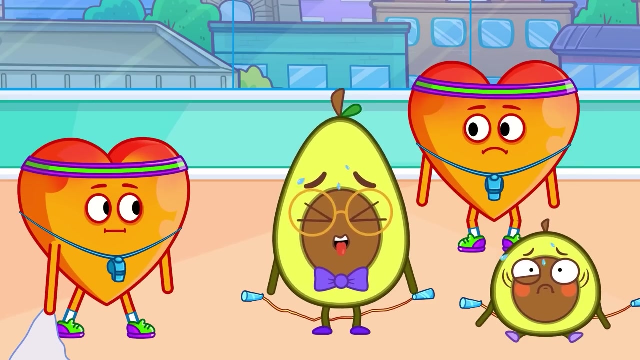 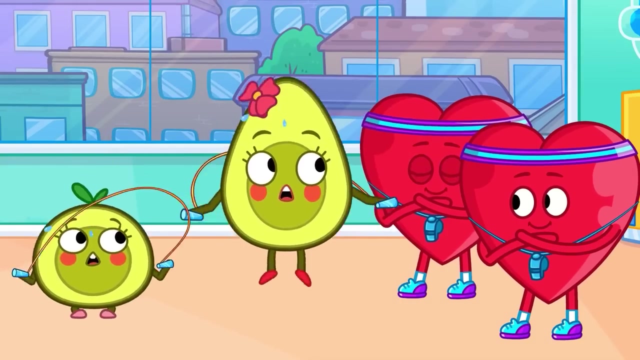 The boys are eating pizza. Eating salad is good for your muscles, But too much pizza will make you weak. Pit and Daddy are now exercising, Just like Mommy and Penny. Let's go faster. Oh no, The boys are too tired to jump rope, But the girls are full of energy. 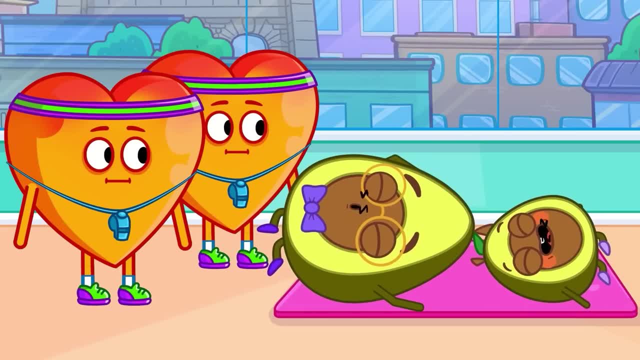 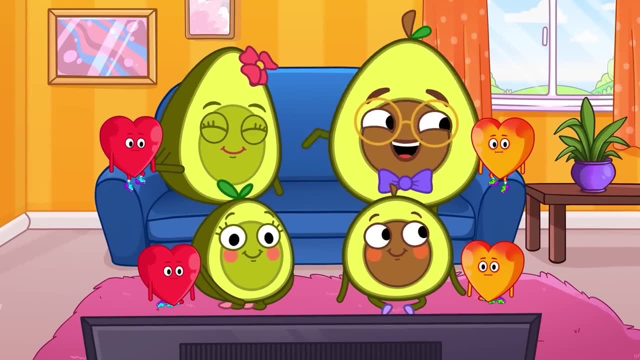 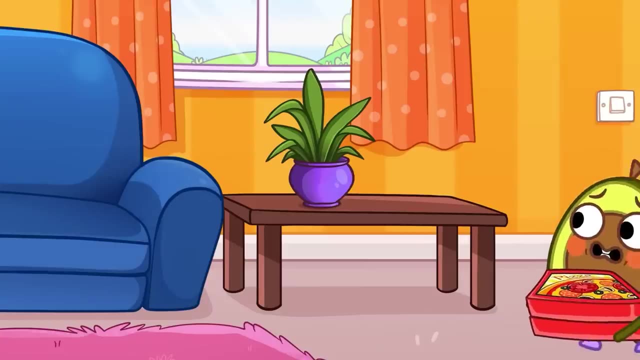 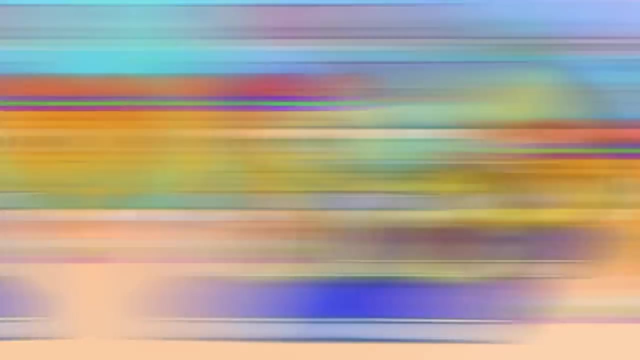 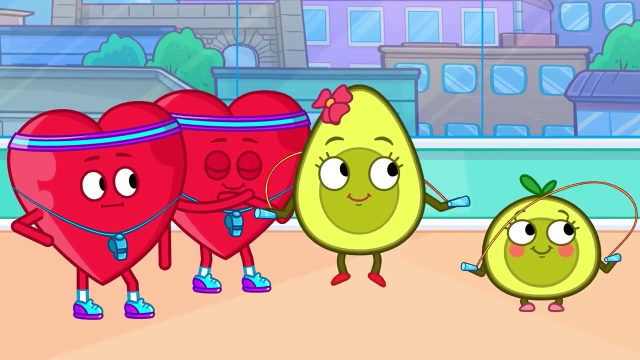 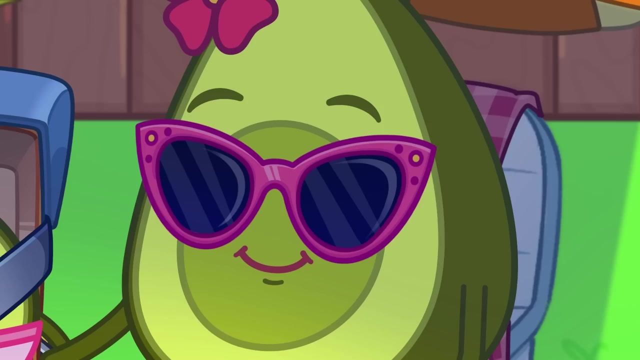 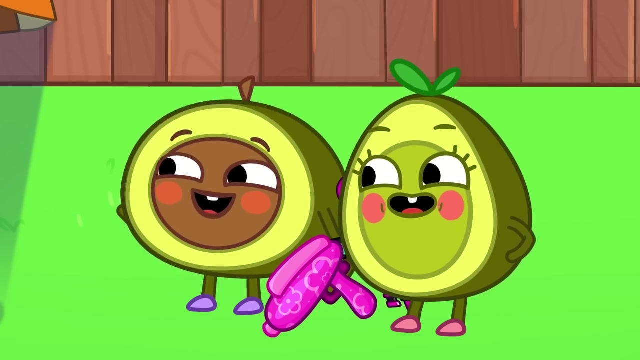 Mommy, you should check on them. Check on Pit and Daddy. They've fallen asleep. Dinner's here, Pit, that looks very heavy. Good thing, the girls exercise. You can do it, boys. You're getting strong already. Hmm…, Hit and Penny are playing with squirt guns. 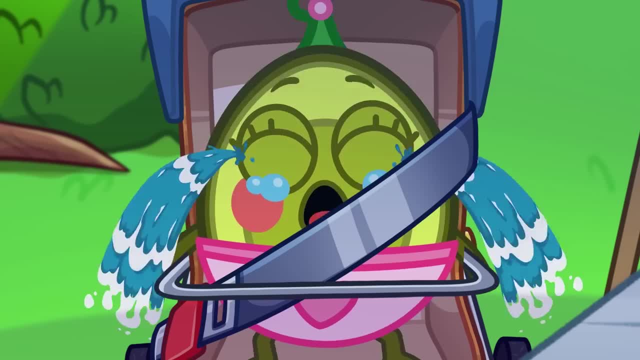 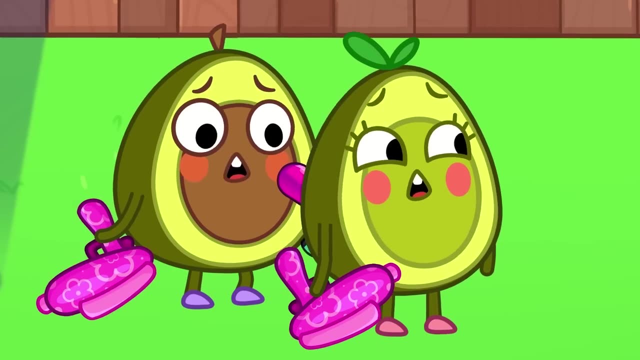 Oops, Mommy just got wet. Good job, Do you want to play too? Hit and Penny are playing with squirt guns. Oops, Mommy just got wet. houette, Do you want to play too? Mommy wants to play as well. Sorry, Kids. 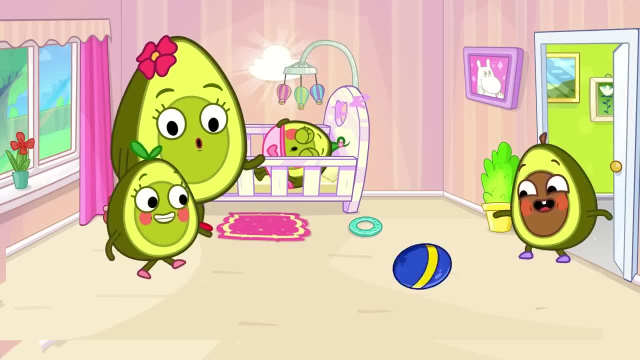 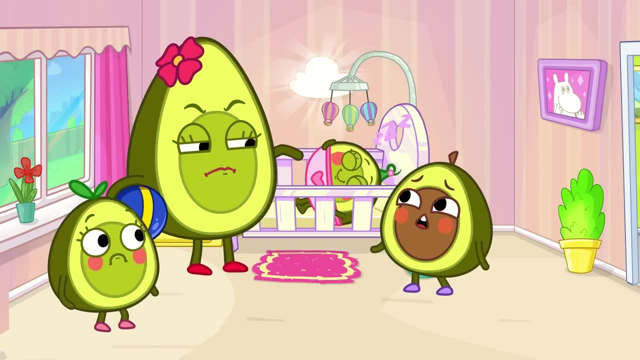 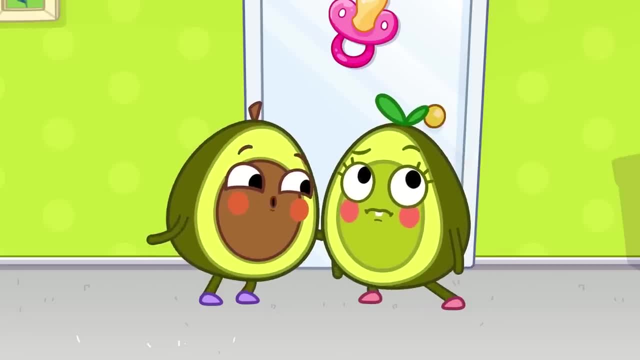 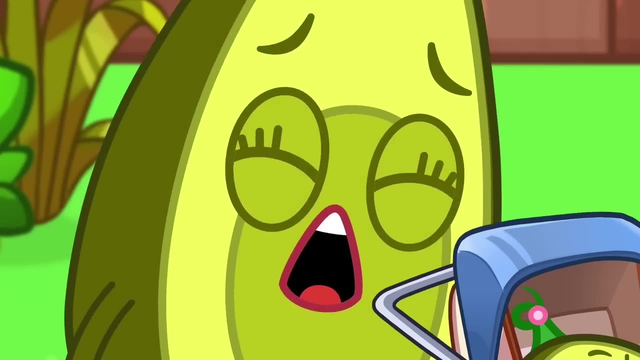 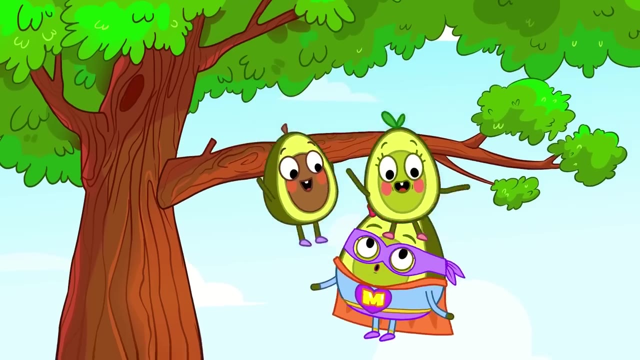 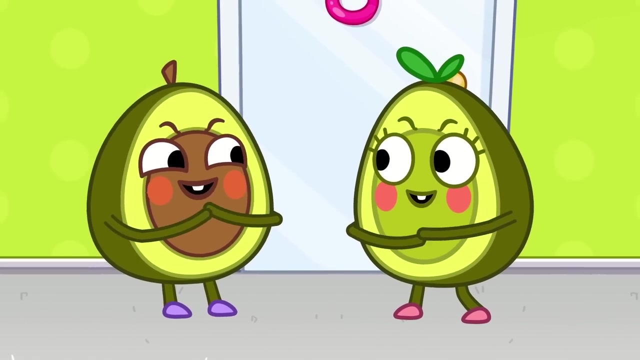 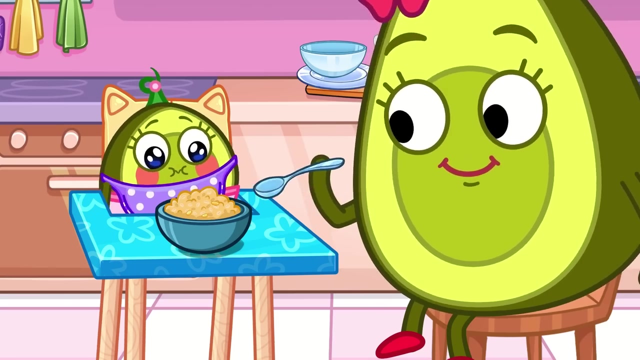 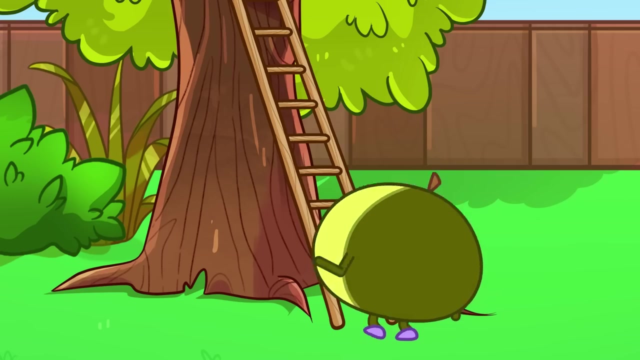 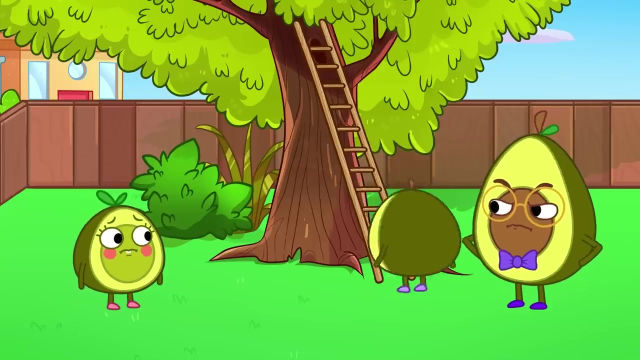 But Pit has an idea. Mommy, help us, Super Mommy to the rescue. I don't know if that's such a good plan, Pit. This plan could be dangerous. Here comes Daddy. He doesn't want Pit and Penny climbing the tree. 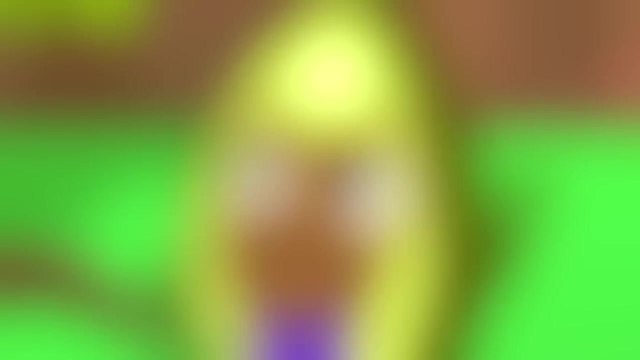 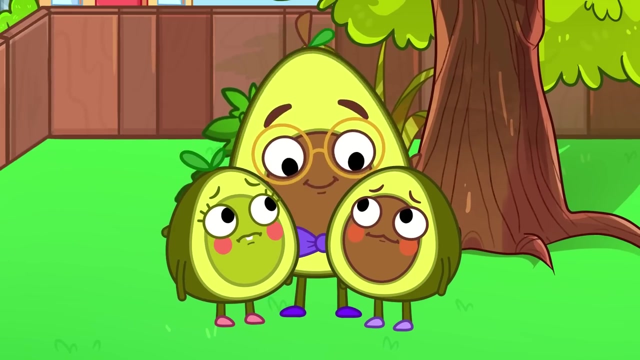 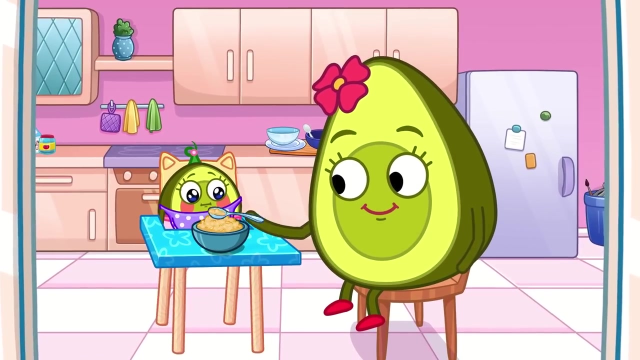 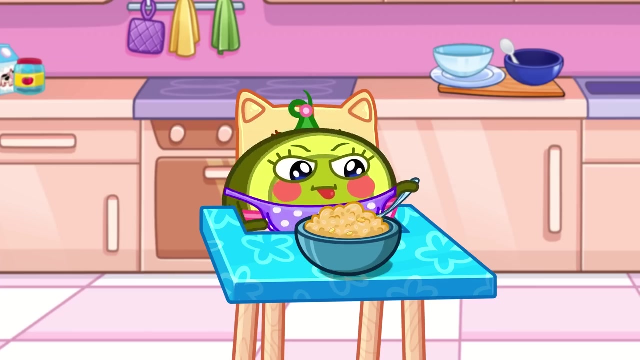 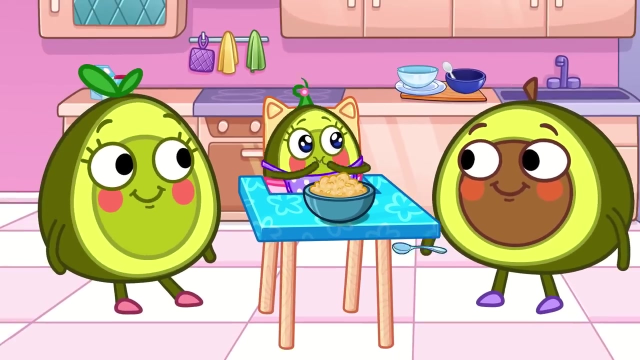 Mommy, help us. We're sorry, Daddy. We feel jealous. Our sister is too small and she needs our care. Baby needs lots of Mommy's help right now. Now you can all spend time together. It's time to clean up the room, Pit. 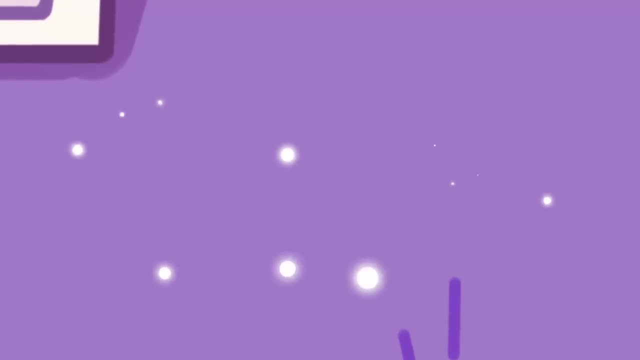 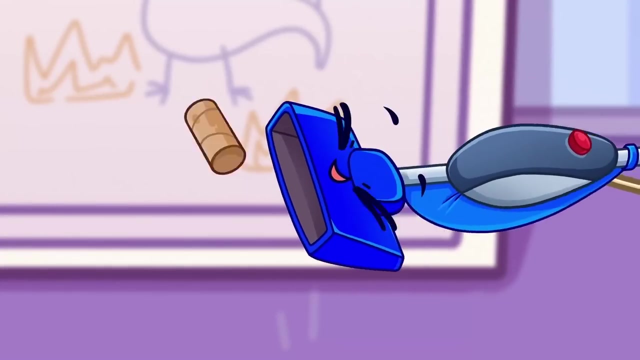 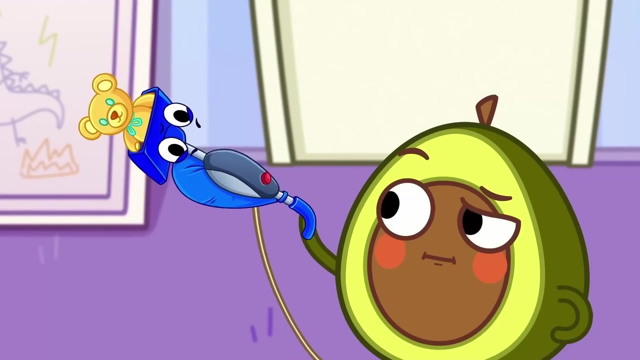 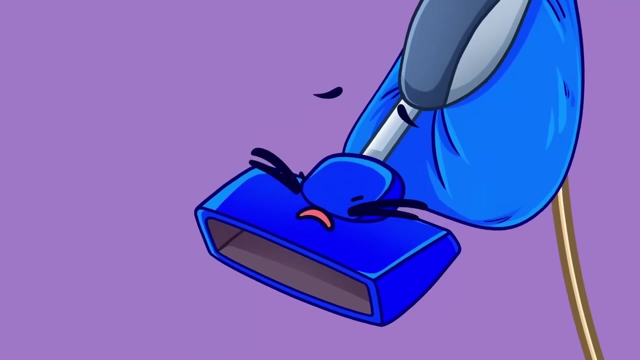 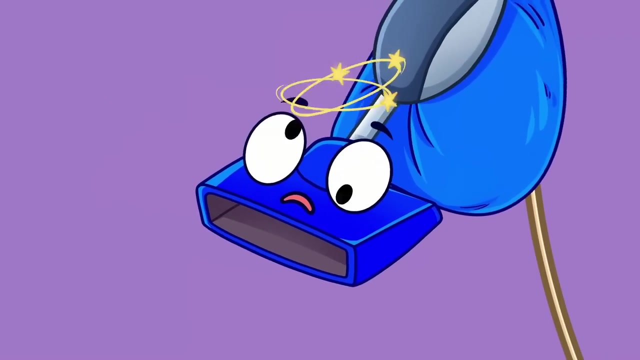 The vacuum cleaner is a great idea. It's a great tool, But it's only meant for small things. That teddy is too big. Now it's clogged. It's time to clean it up. It's time to clean it up. 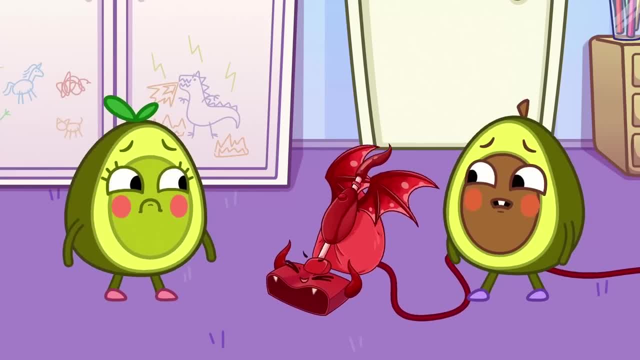 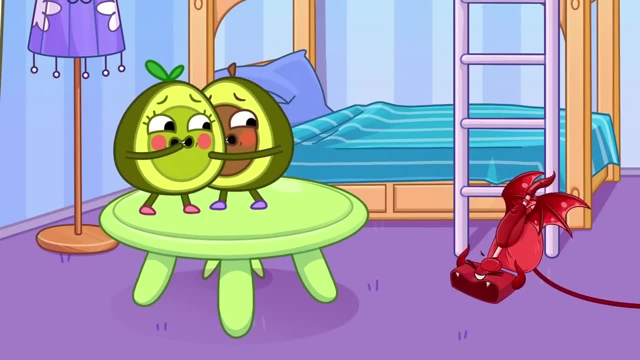 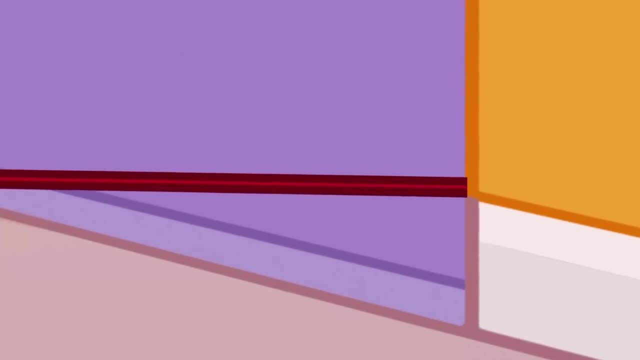 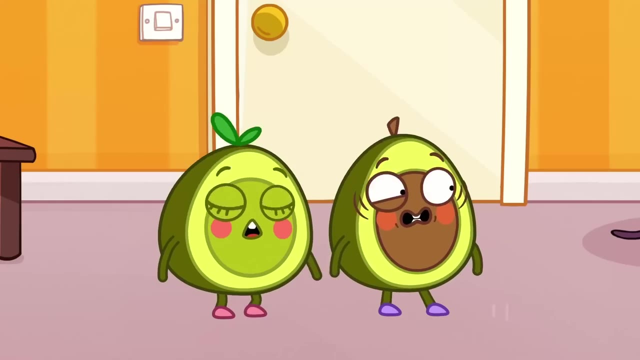 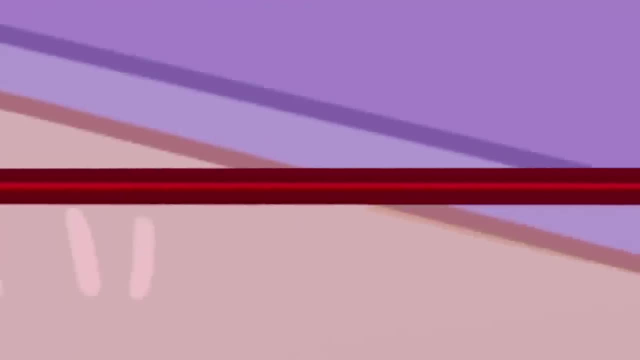 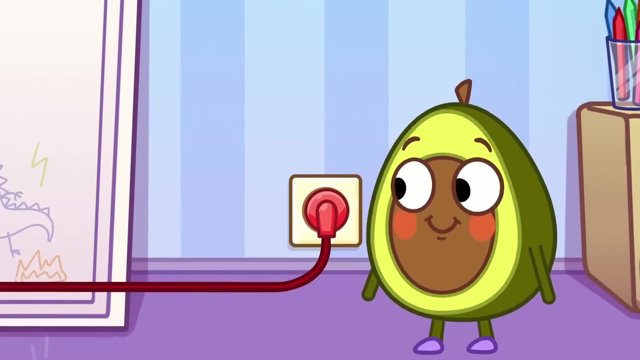 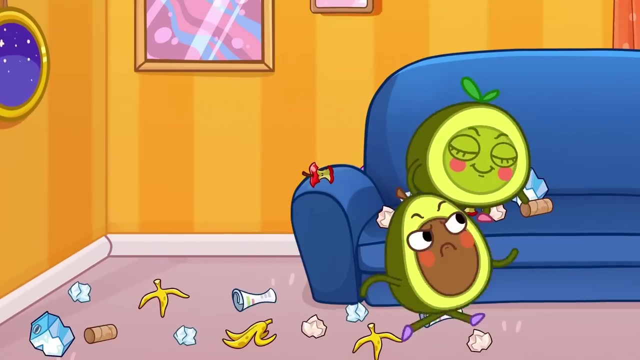 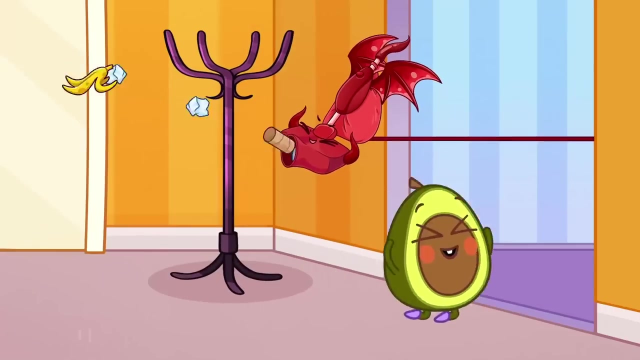 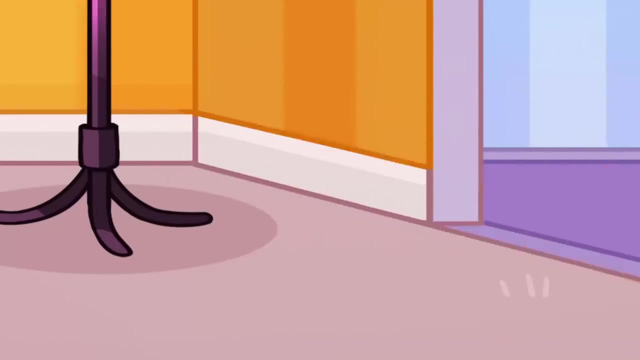 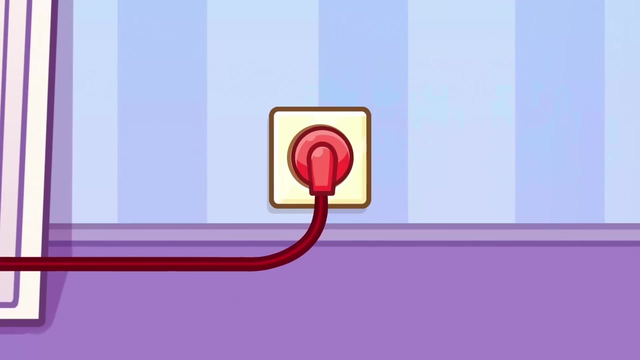 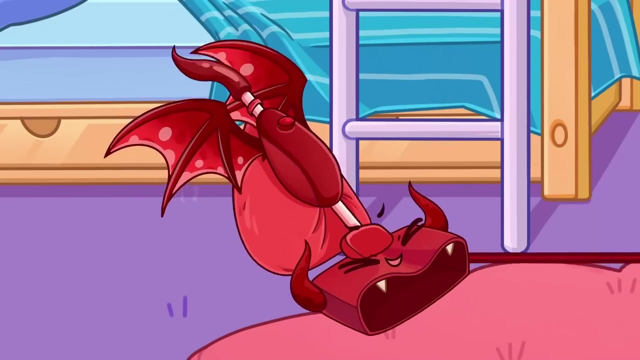 Look, It is powered by a cord To defeat the vacuum. Pit wants to unplug it. Penny will distract the vacuum And Pit will pull the plug. Hurry, Pit. You did it. It didn't work, But why? 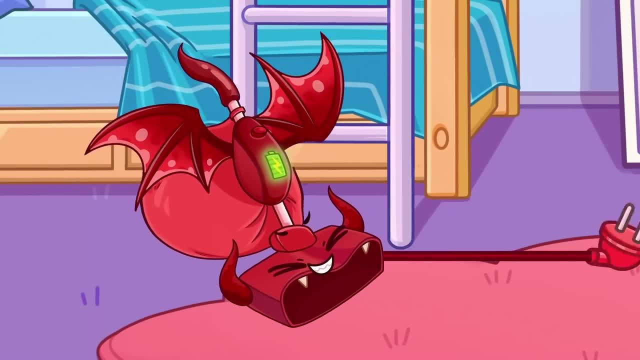 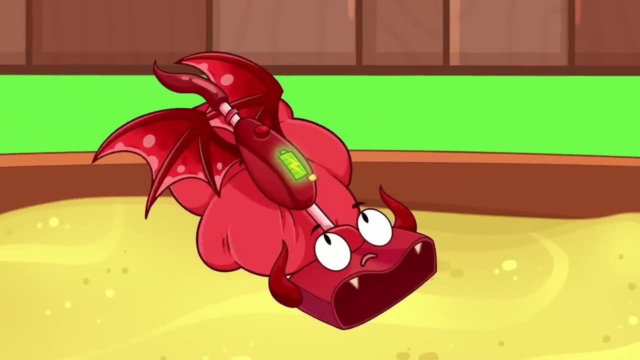 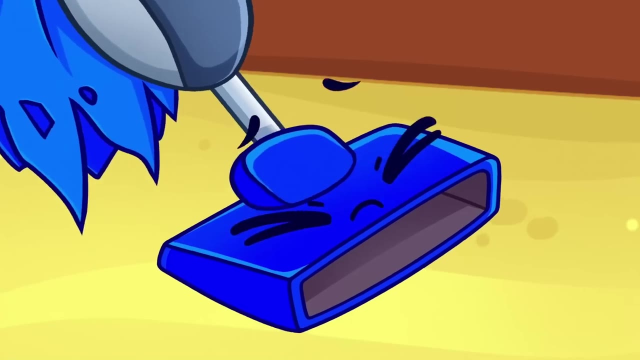 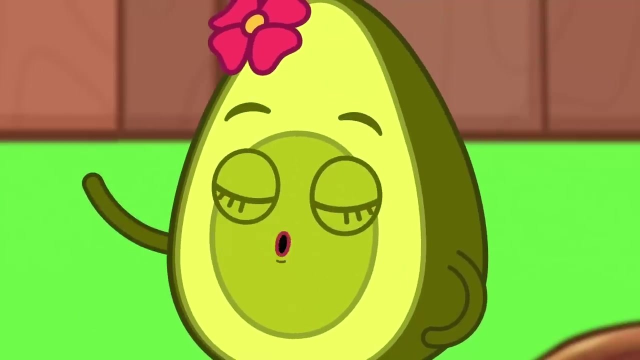 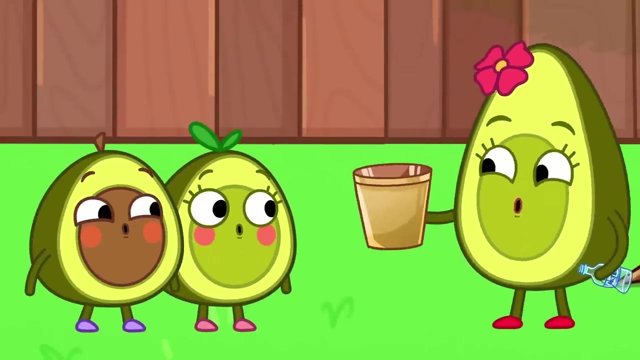 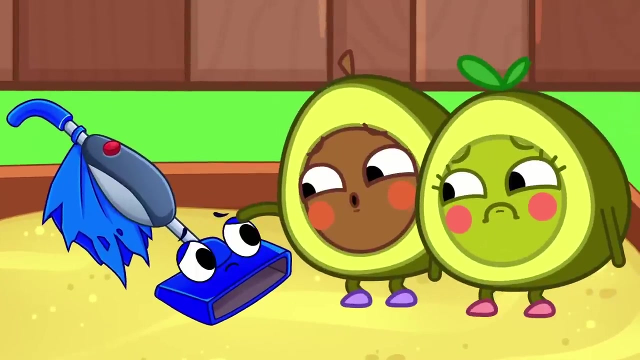 I have a fully charged battery. The vacuum is broken. You've been mistreating me. What, What, What? The vacuum cleaner must be used correctly. Large rubbish should be thrown into the bin. We're sorry. We will take care of you. 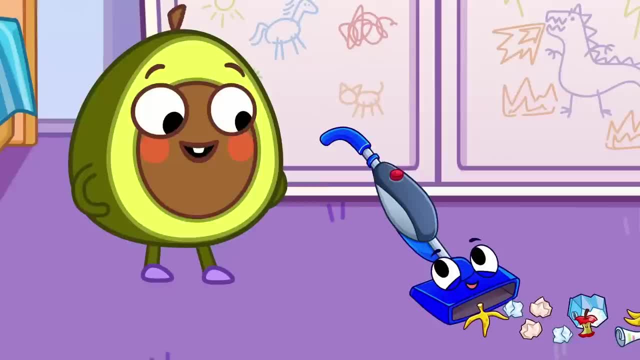 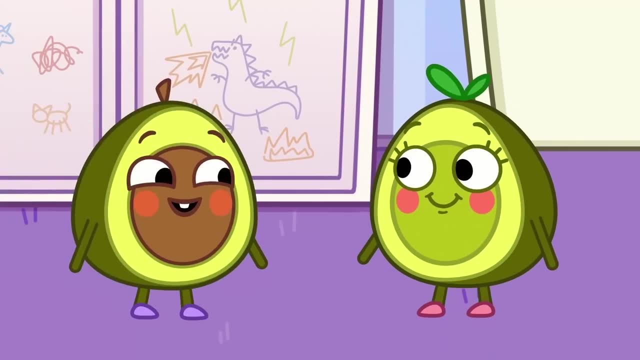 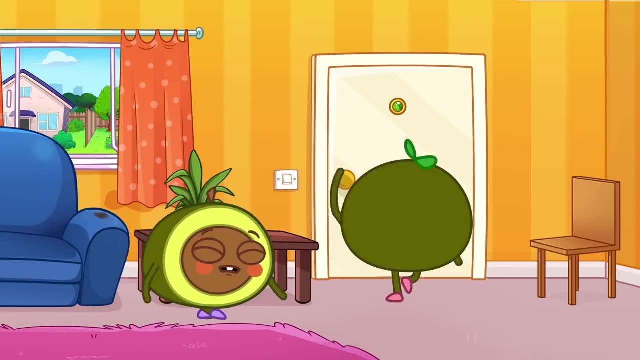 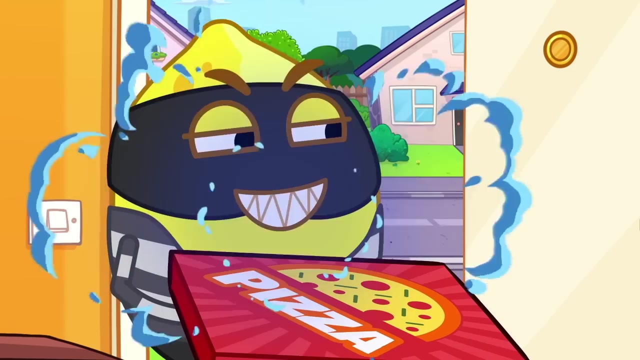 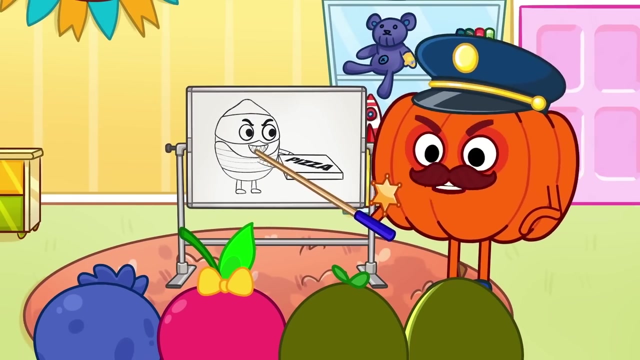 Remember Big pieces go in the trash And small pieces go in the vacuum. Wait, Well done kids. Someone's at the door. Who's there? Pizza delivery- I love pizza, Mr Lemon. Never let strangers into the house. 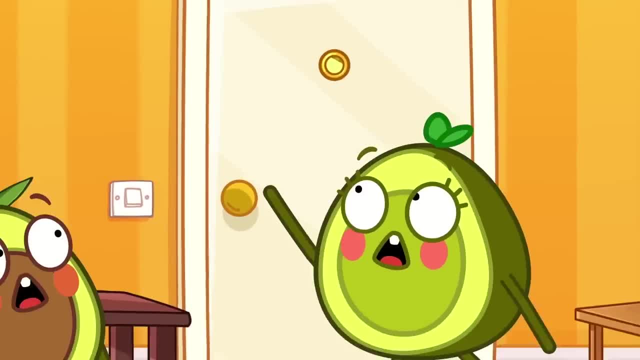 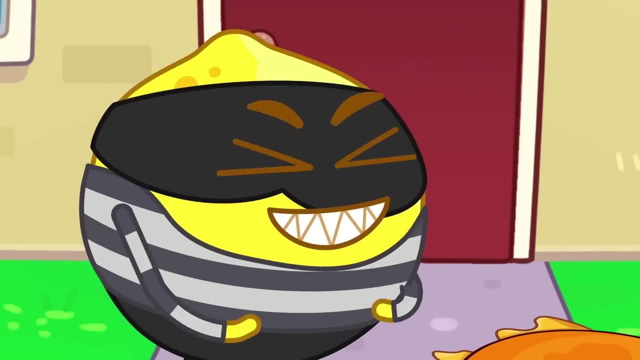 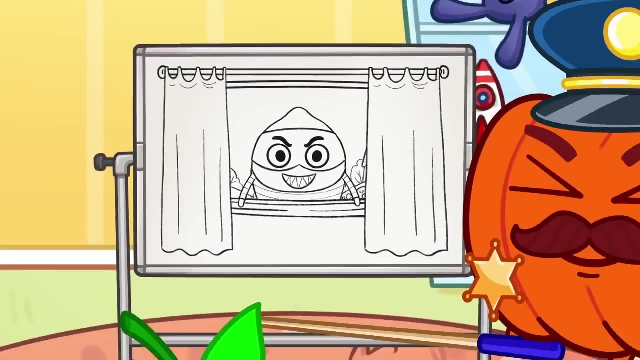 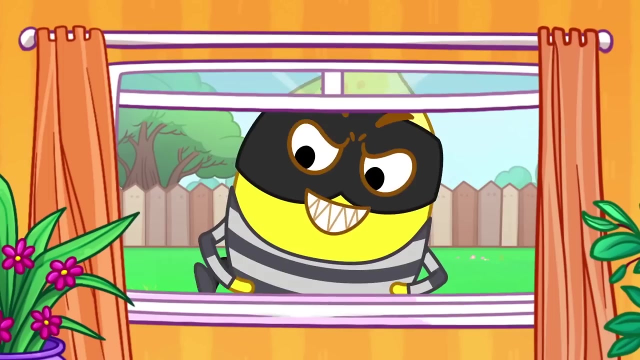 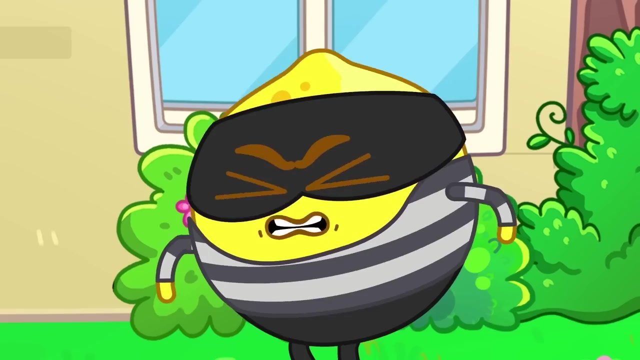 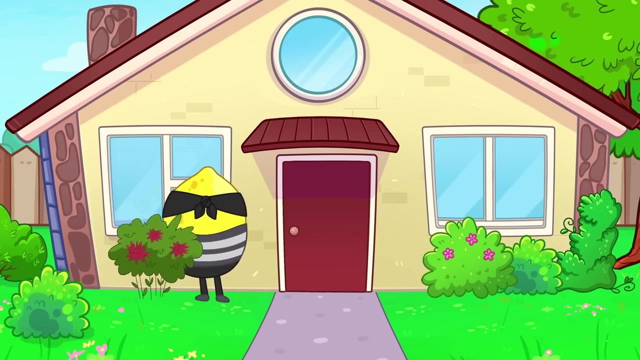 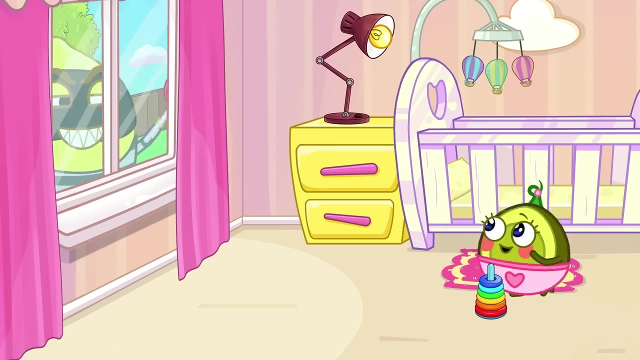 Oh Hahaha, Go away. What if he tries to get in the window? If you see a stranger, lock all the doors and windows. That was close. Oh no, He's going to trick Baby And Baby, let him in. 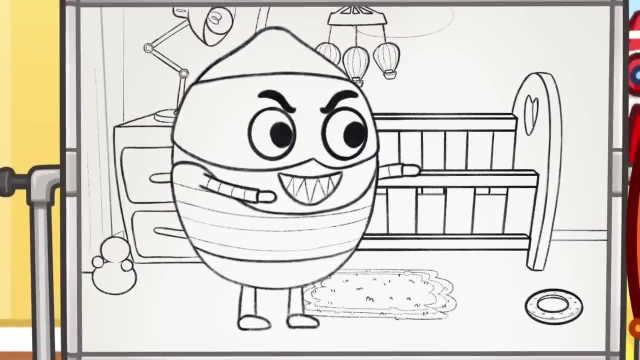 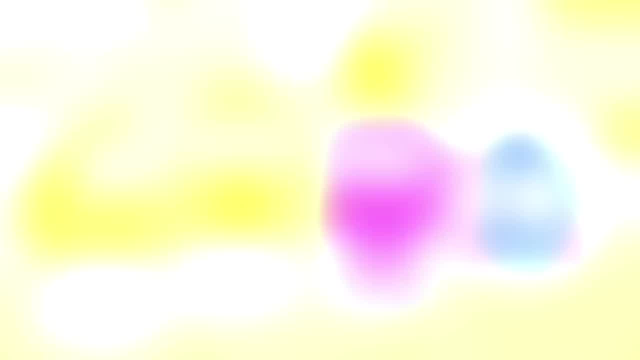 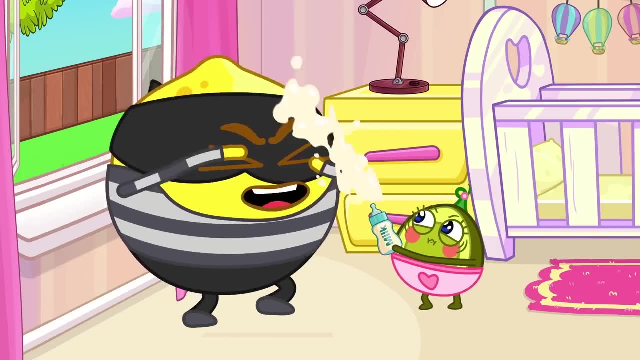 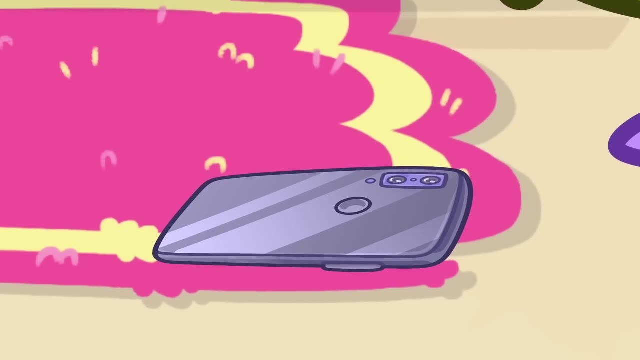 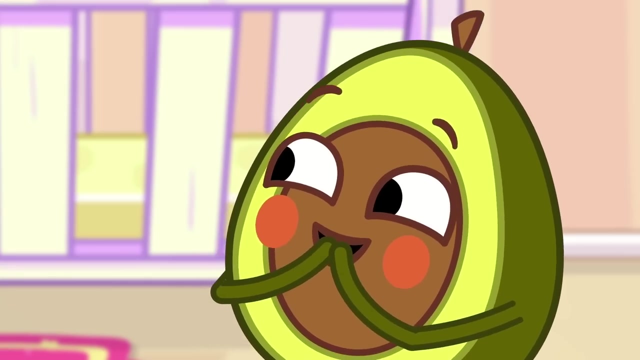 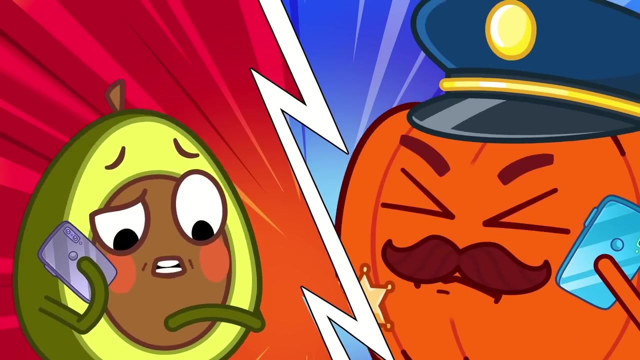 What should we do now If a stranger breaks into your house? call 9-1-1-8!. Immediately, Come with me, Baby. Call 9-1-1,. Pitch, A stranger has broken into our house. This will slow him down. 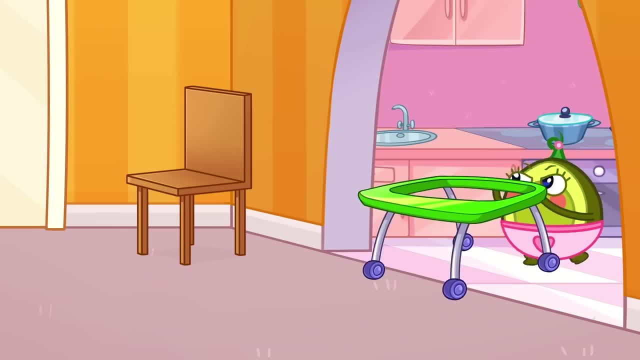 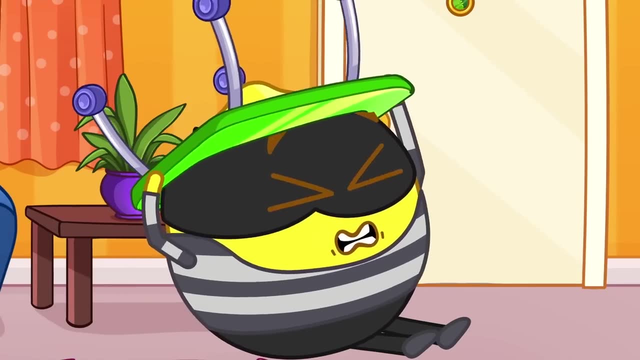 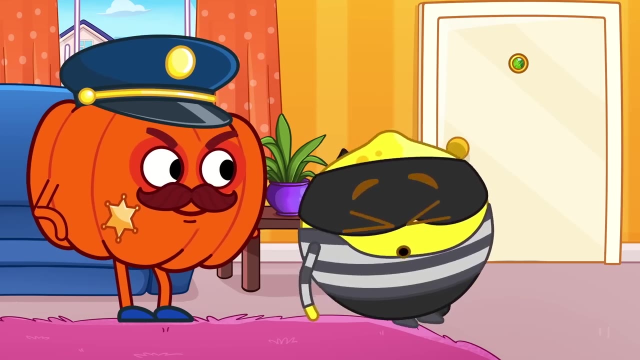 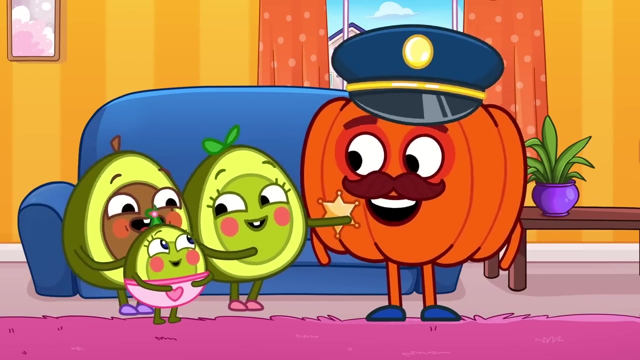 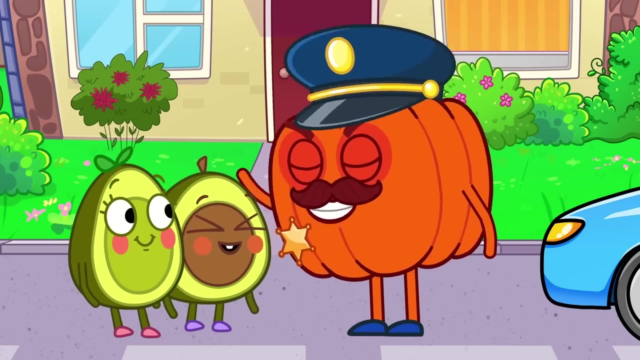 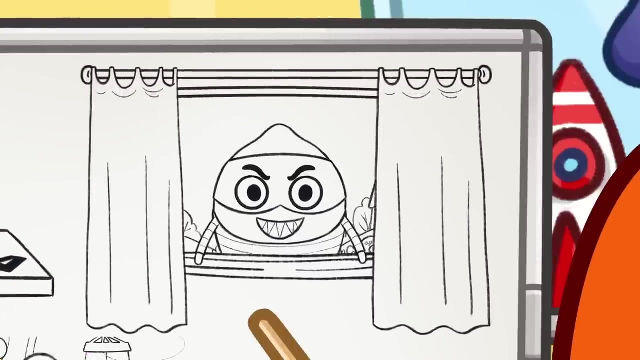 Oh my God, Officer Pumpkin is here. Call 9-1-1-8! Well done. Calling the police was the right thing to do. Don't open the door to strangers. If you see a stranger, close all the doors and windows. 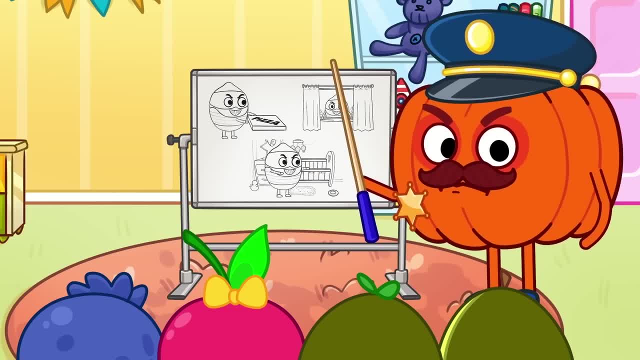 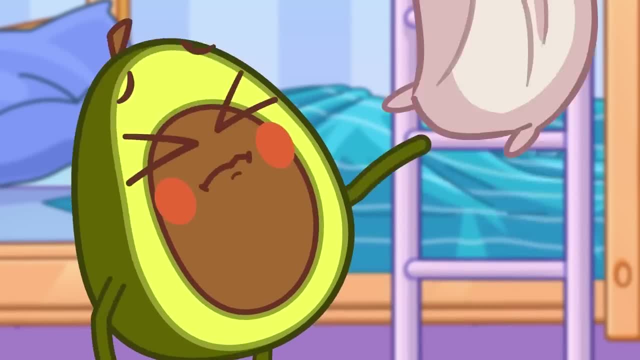 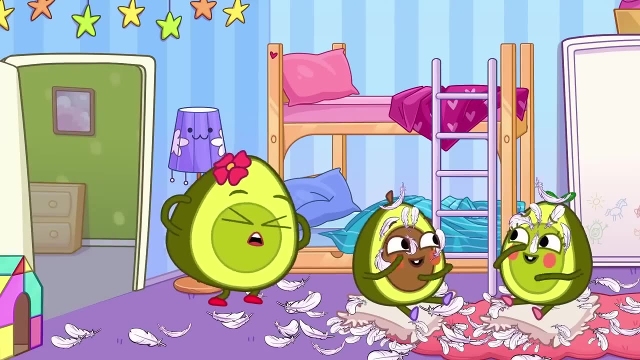 If a stranger is in the house, call 9-1-1!. Thanks, Officer Pumpkin. Pit and Penny are having a pillow fight. Oh no, Look at the mess you made. Mommy doesn't seem very happy about it. 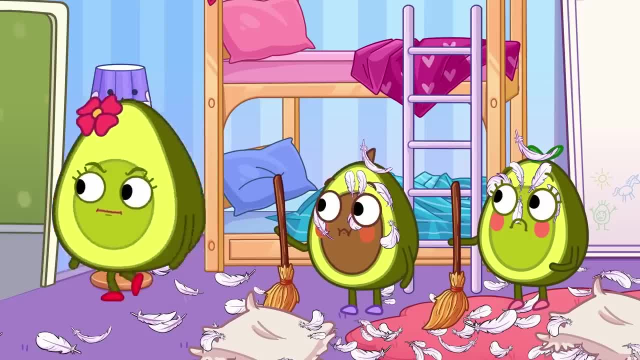 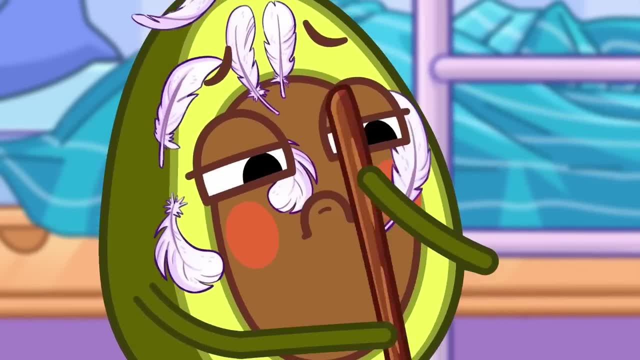 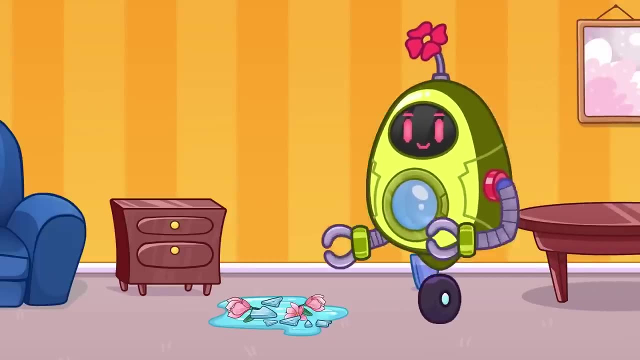 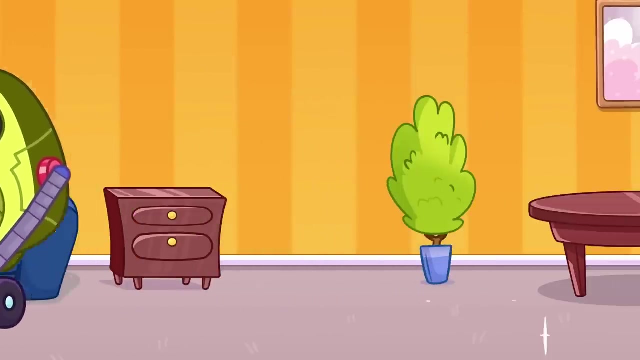 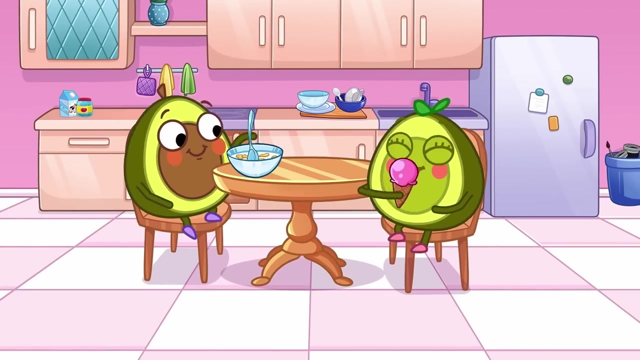 You two need to clean up this mess. I wish I had a robot Mommy. Let's imagine what that would be like. A robot Mommy would clean up all your messes. Uh, oh, Oh, Oh, Oh, Penny. 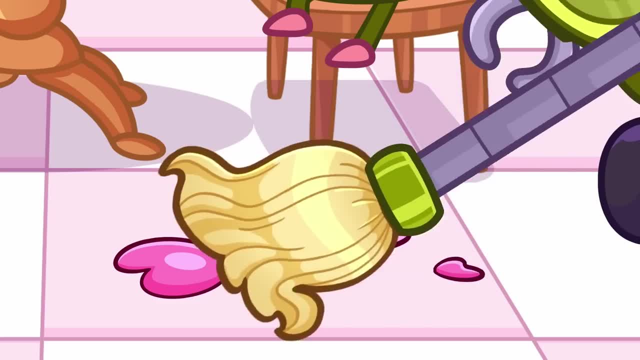 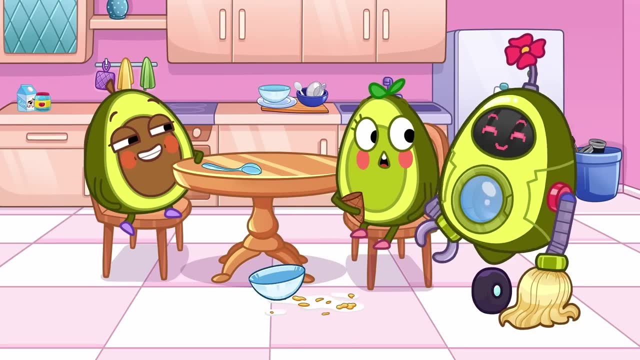 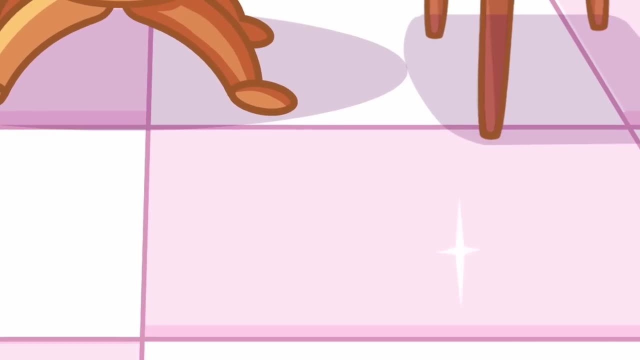 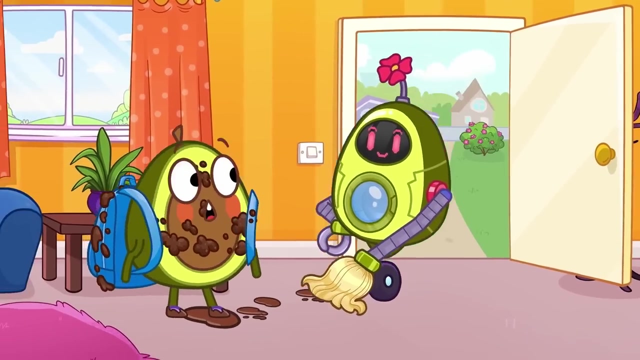 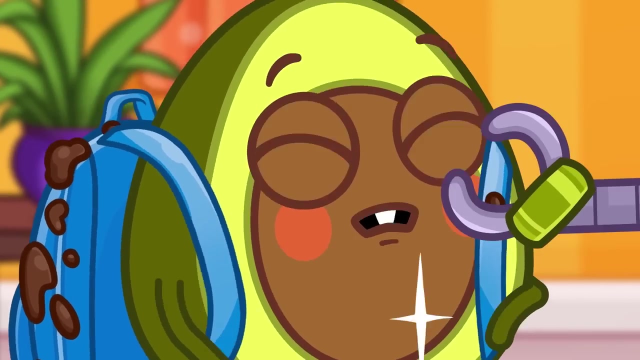 You dropped some ice cream. Uh oh Robot, Mommy can handle it. Now Pit is making a mess on purpose. Oh Oh, Oh. Oh Wait, Pit, You're covered in mud. That's better, Your backpack is clean too. 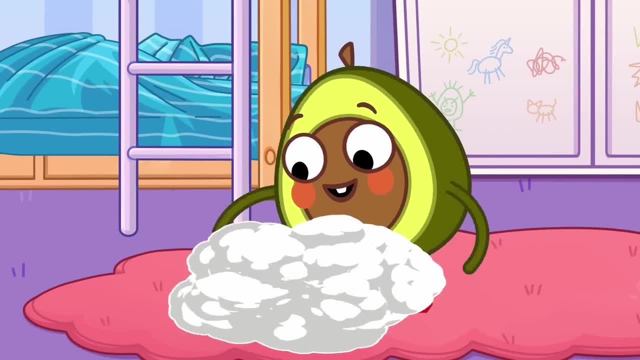 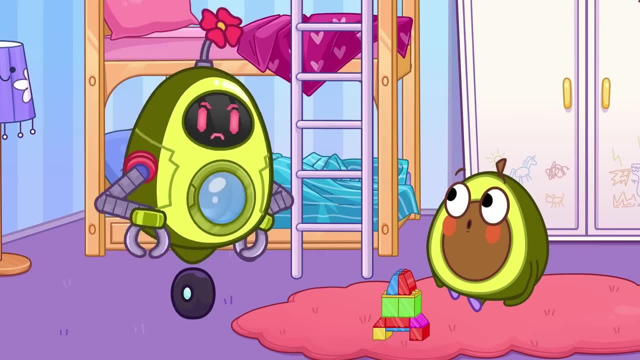 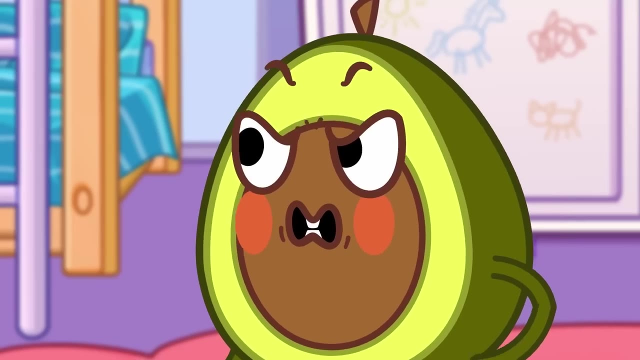 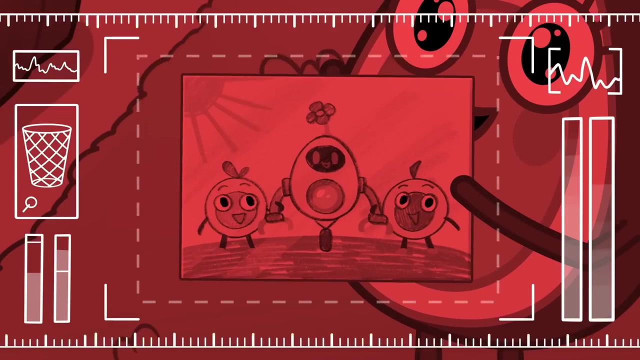 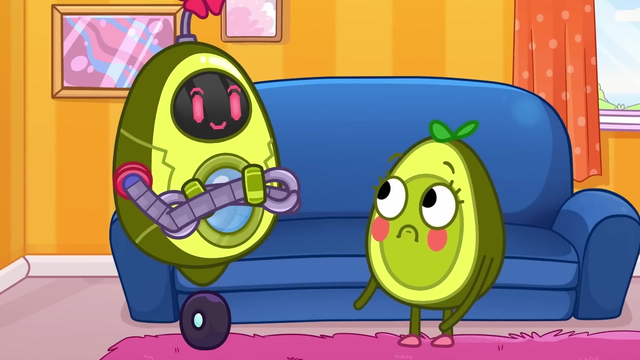 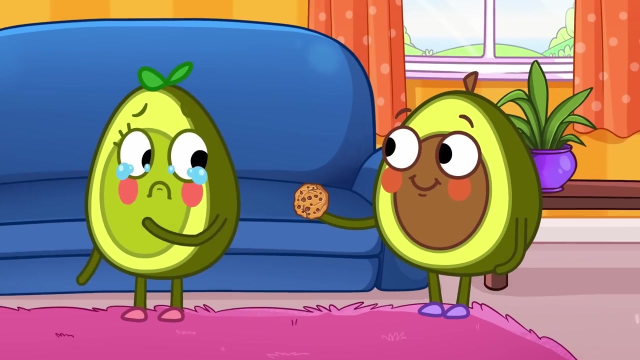 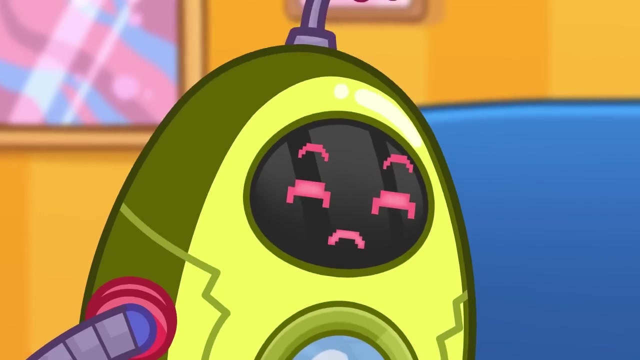 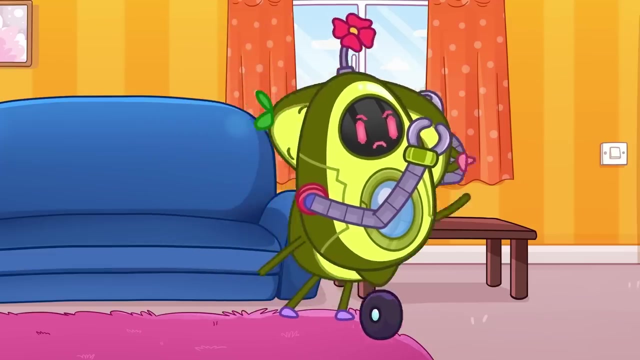 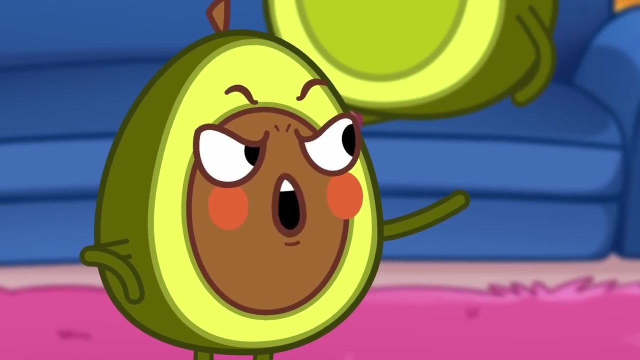 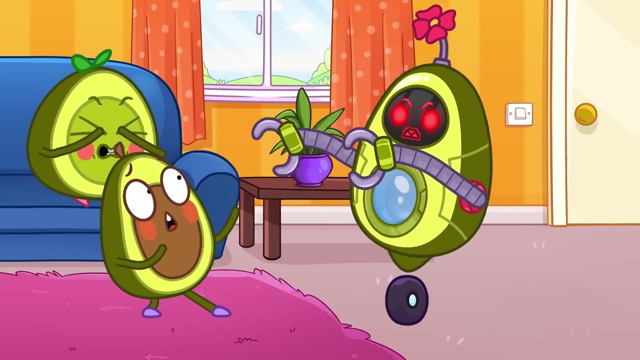 But Robot Mommy thinks your toys are trash And Robot Mommy thinks your art is trash as well. Watch out Penny, Help her Pit. You are not my mom. Robot Mommy, Robot Mommy looks angry. Good thing she isn't real. 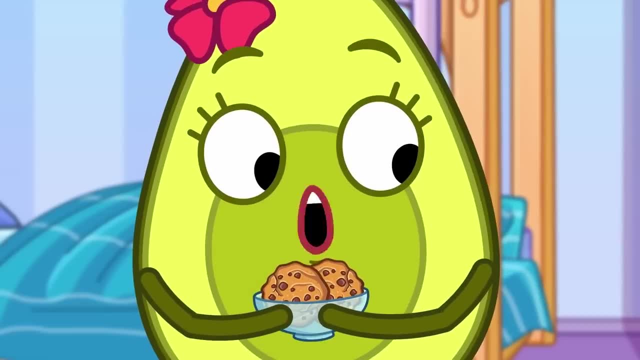 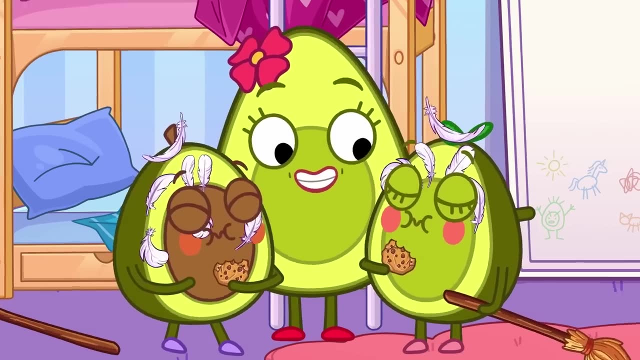 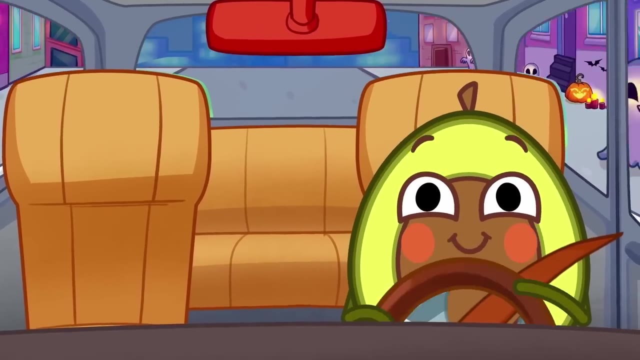 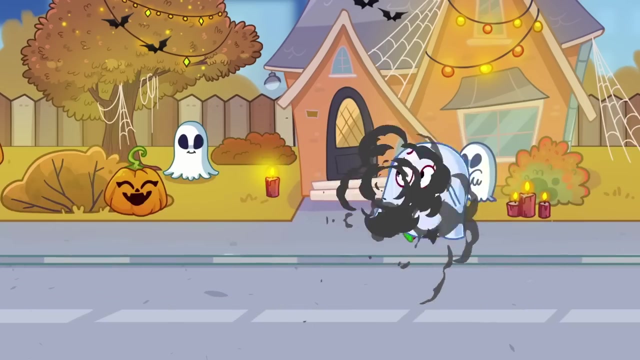 Look, it's real Mommy For my little helpers. What do you think, kids, Our Mommy is better than a robot. Pit's driving a taxi. Pit, someone needs your help. It's not a ghost, It's Cherry. 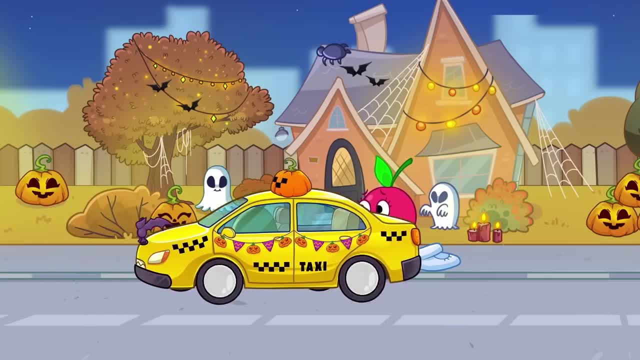 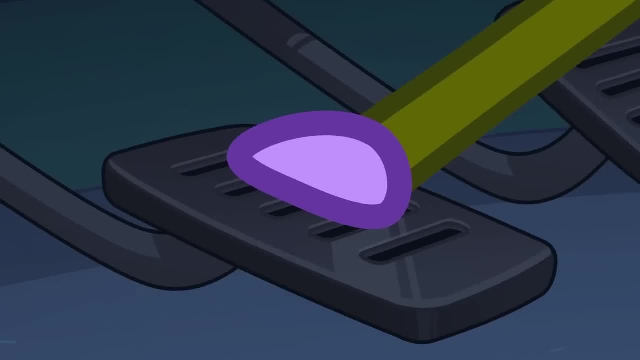 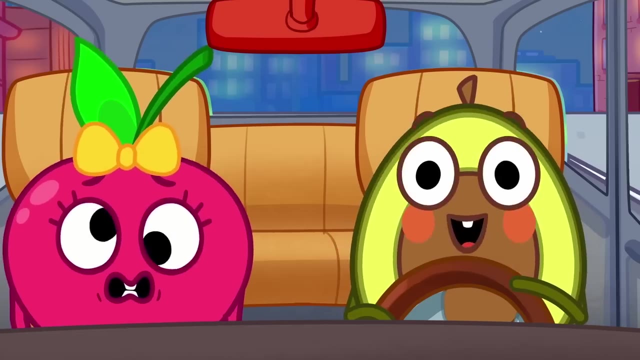 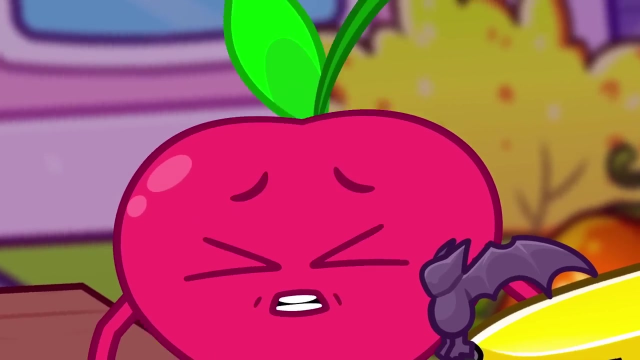 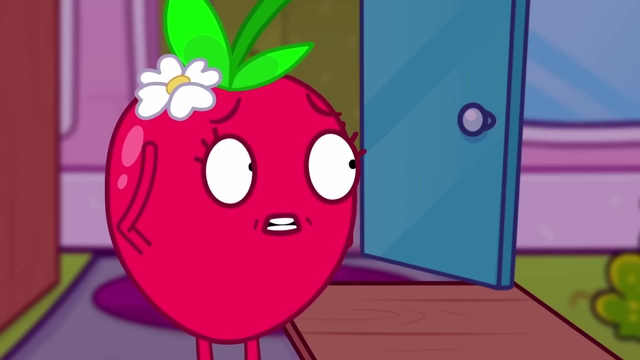 Taxi, Take me home. please, Let's go find your home. Don't drive too fast, We've arrived. We've arrived Now, Cherry's dizzy. Don't go, My little friends, Don't worry, Pit will fix it. 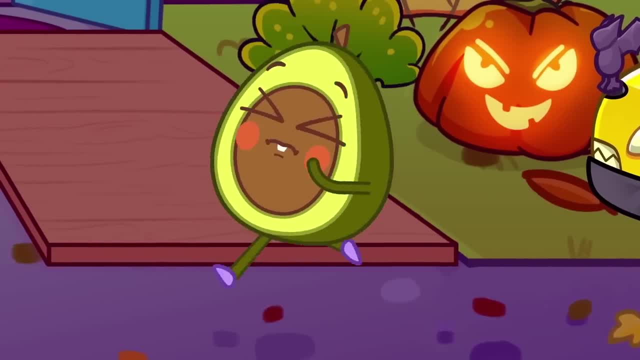 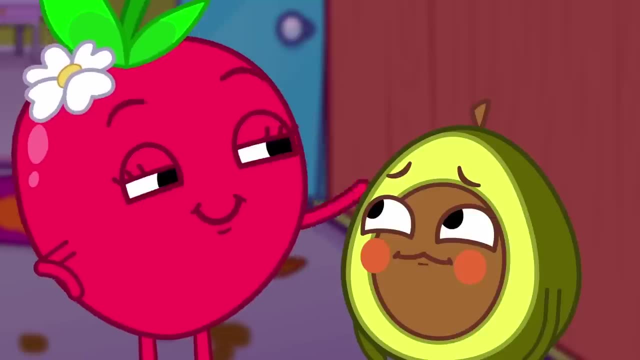 Don't worry, Pit will fix it. jonk, I'm so sorry, I'll be careful. Thank you for breeding Cherry home. I didn't ask to You saved me. Thank you, baby, You helped me, Hihi. 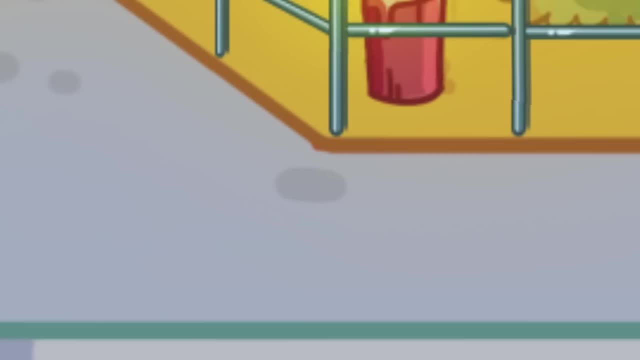 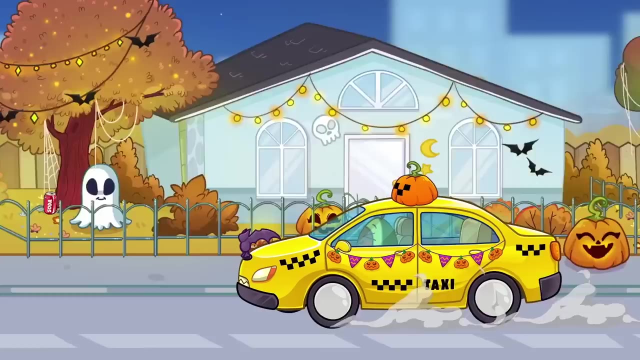 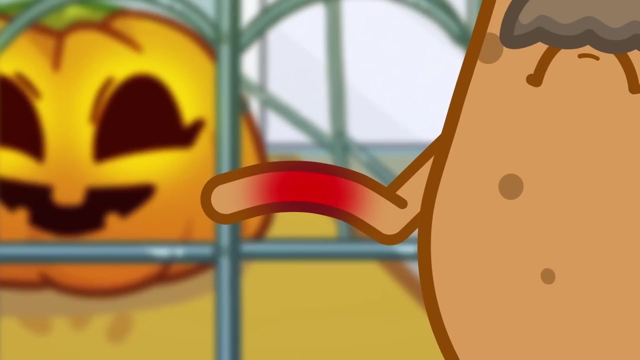 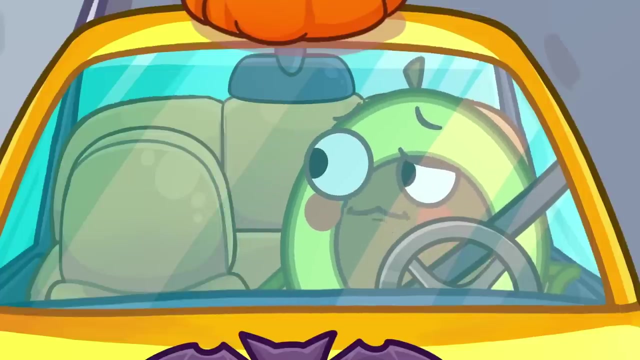 You saved me. Hahahaha, Pit, that's not where your trash goes. Watch out, Are you hurt My arm? I can take it to the hospital. I'm sorry. I won't let her on the road anymore. That belongs in a garbage, can. 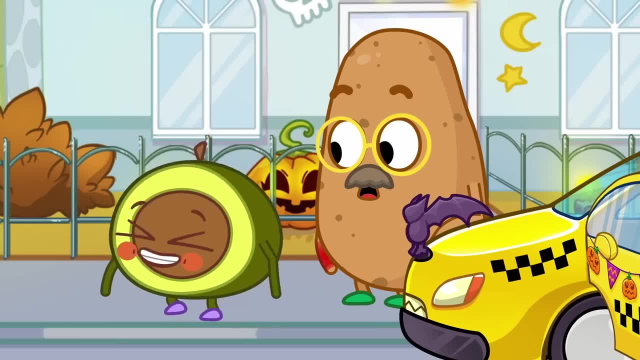 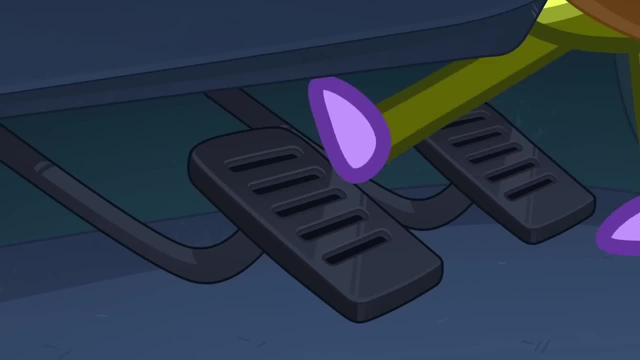 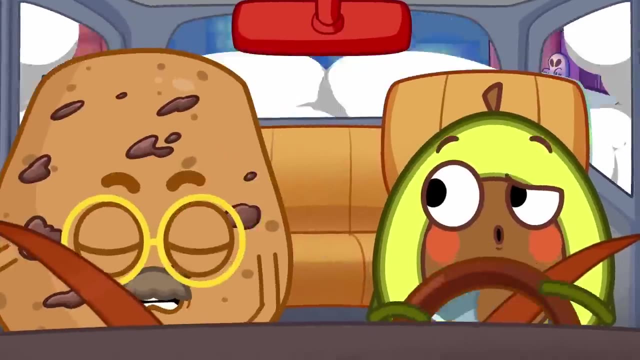 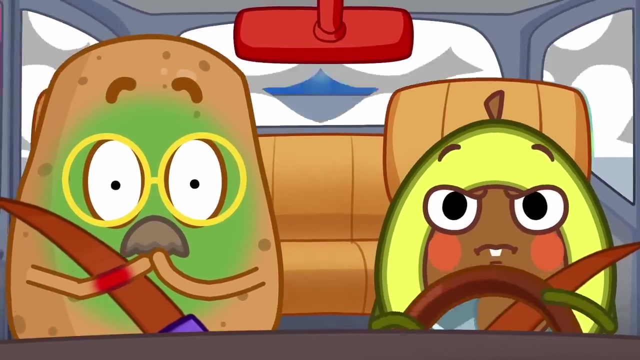 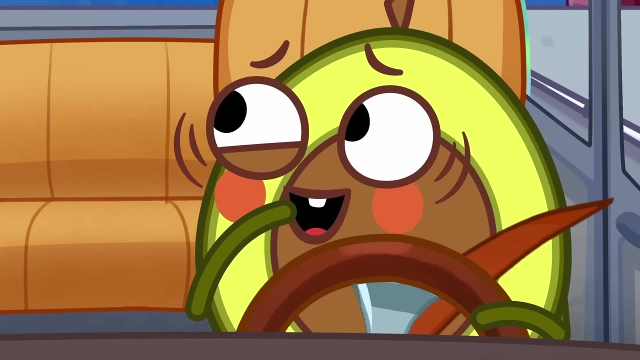 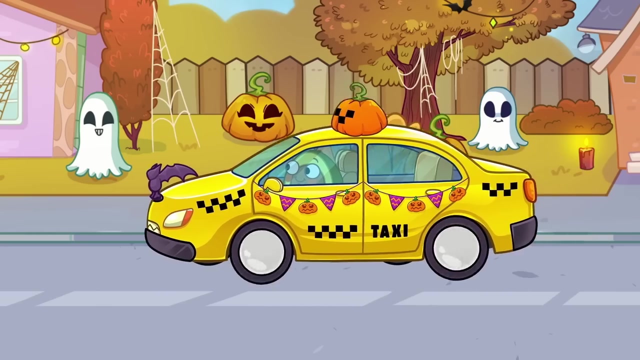 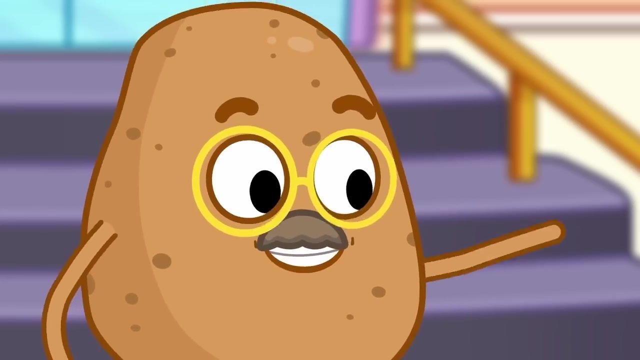 Now let's take Potato to the hospital. Slow down, Pit. You're not driving safely. Slow down. I'm sorry, I won't drive fast anymore There. You made it to the hospital, Oh no, A spark started a fire. 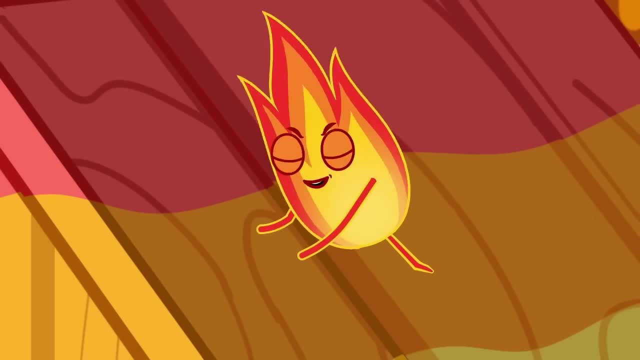 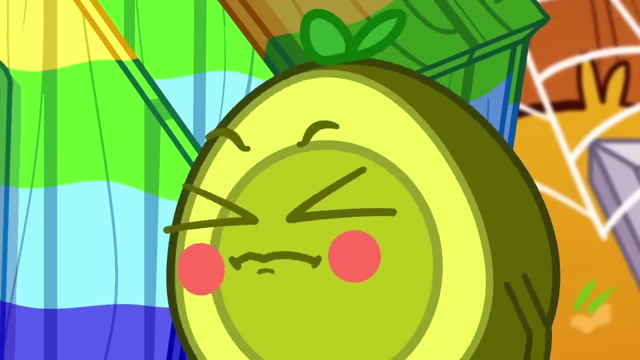 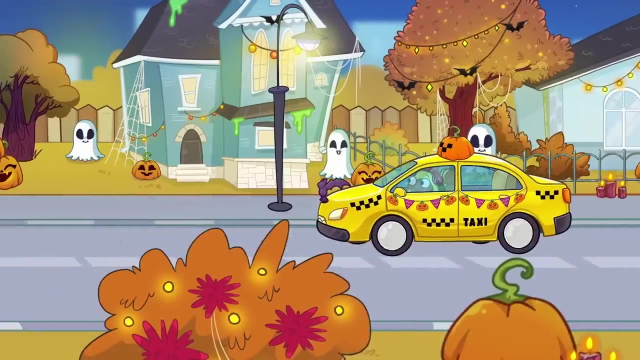 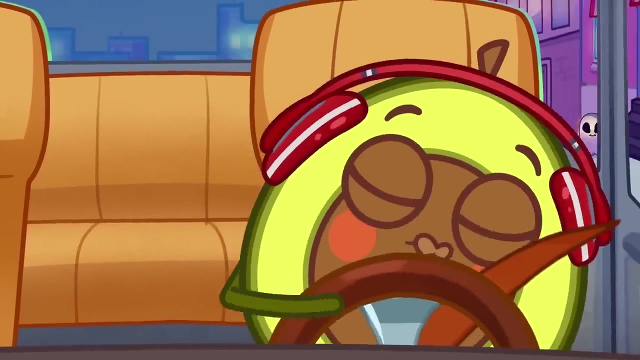 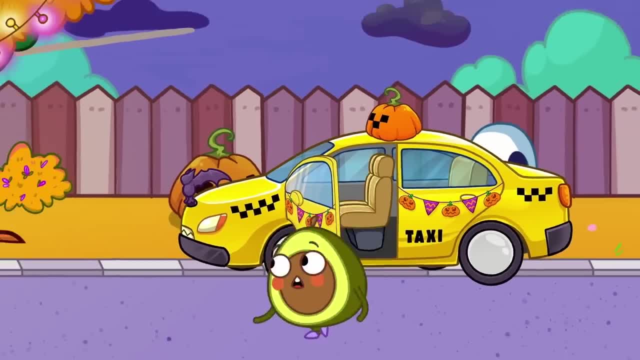 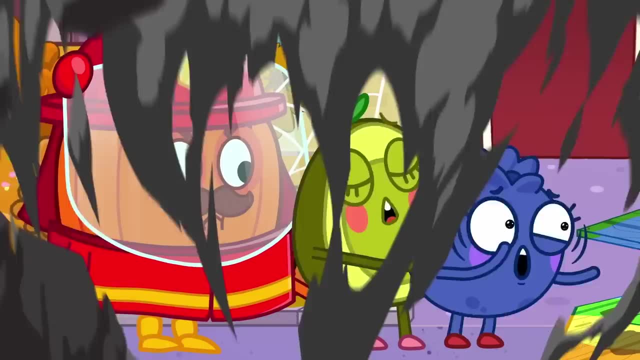 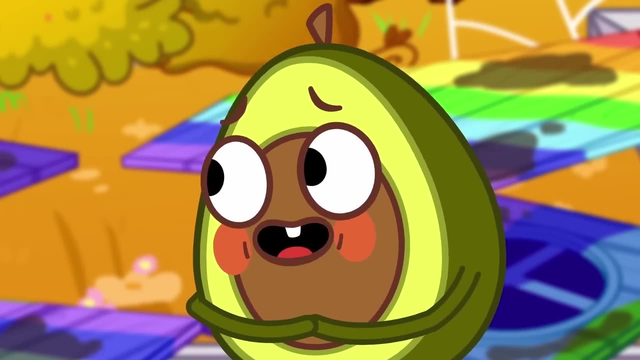 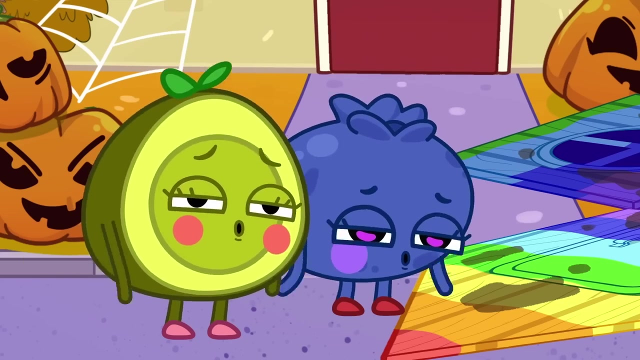 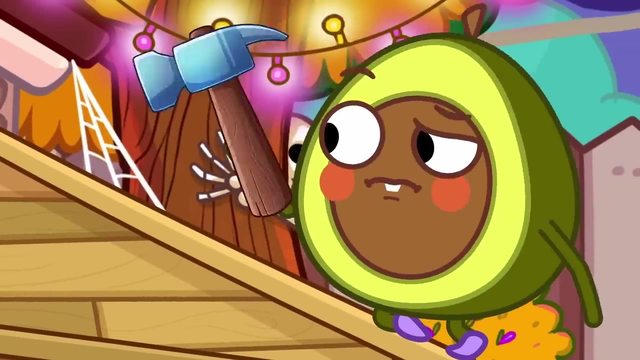 But Pit is distracted and won't get out of the way. Oh, the fort is ruined. You should not wear headphones while driving. I'm sorry, I won't do that anymore. Pit, you need to fix this mess. Good job. 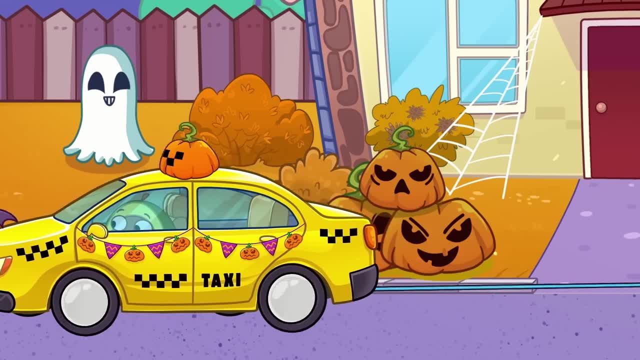 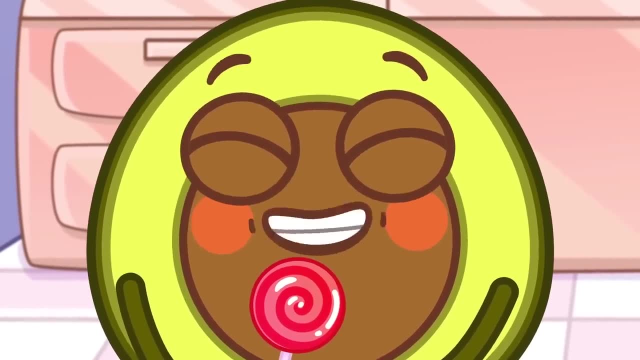 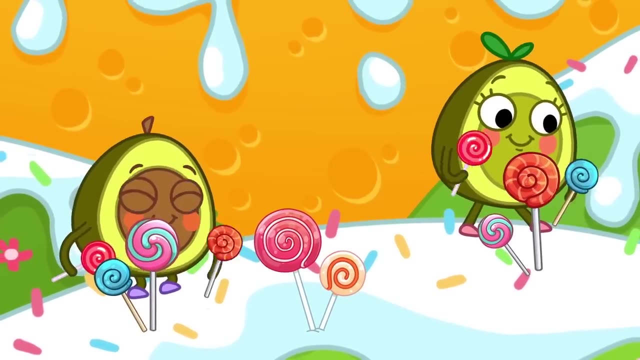 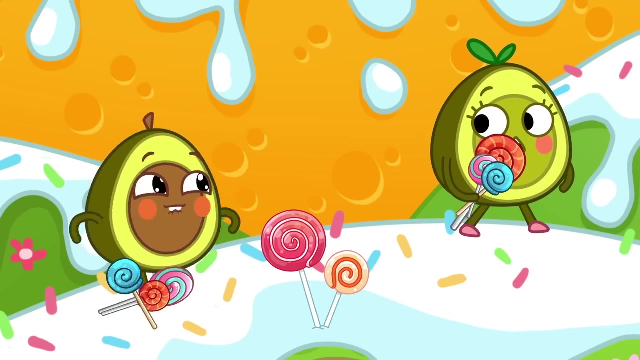 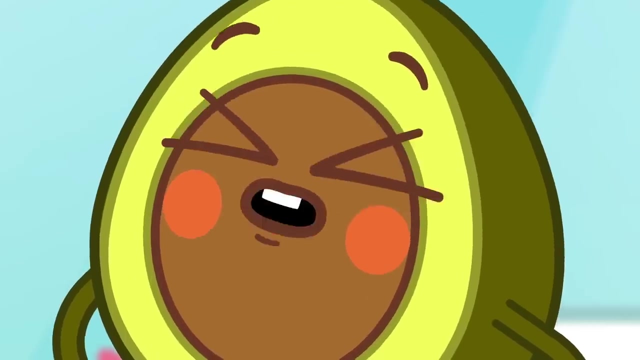 Time for a ride. Have fun, kids. Hello Pit and Penny, I wish I could eat nothing but sweets. Imagine if you lived in a land made of sweets, With lollipop flowers and cotton candy bushes. Look at this, Wow, a candy castle. 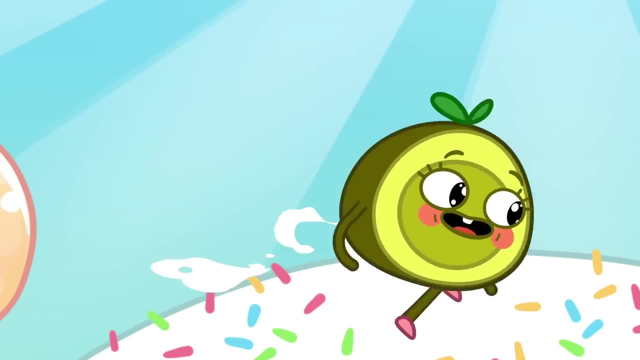 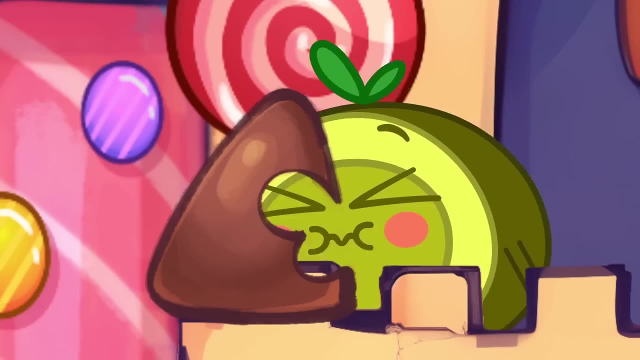 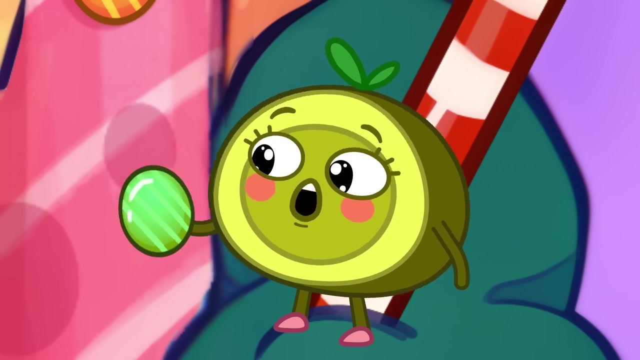 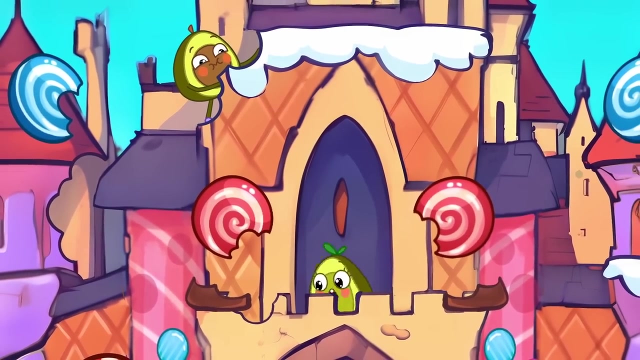 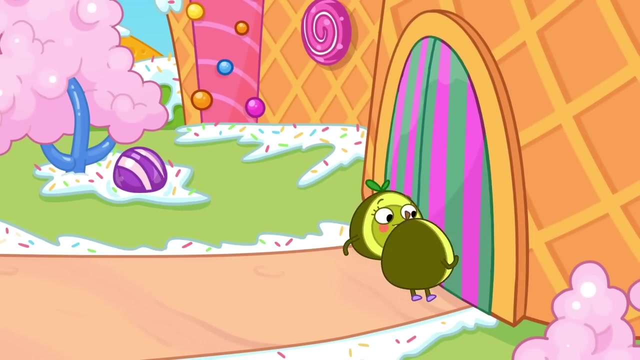 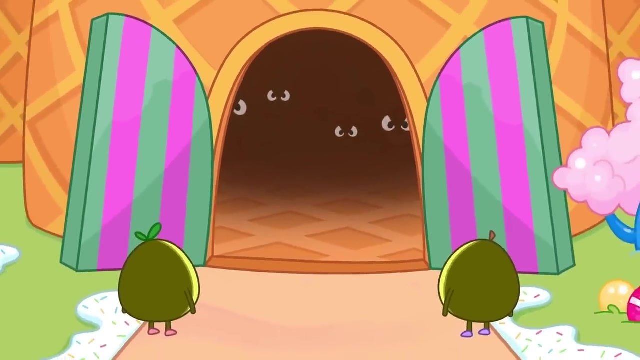 Oh wow, Yummy. Pit and Penny are eating everything in sight, But their teeth are getting dirty. There's a lollipop, Oh no, There's something inside. There's a lollipop Germs, And they love to cause cavities. 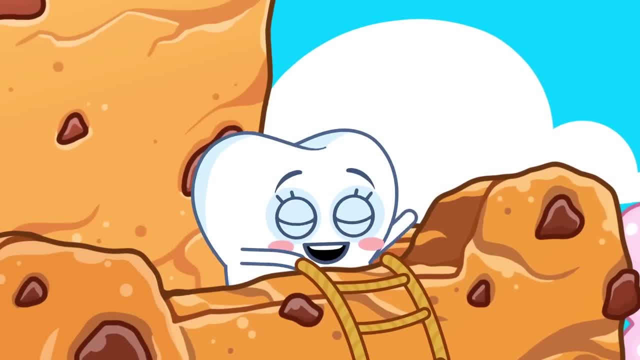 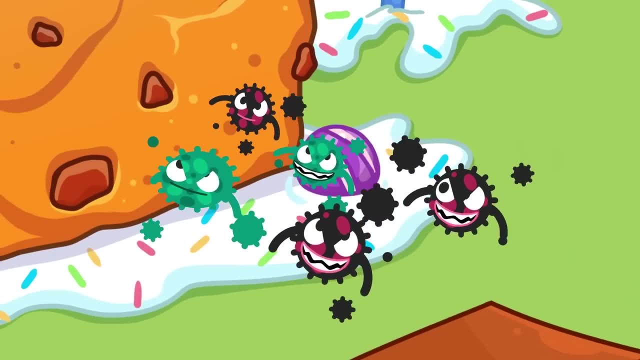 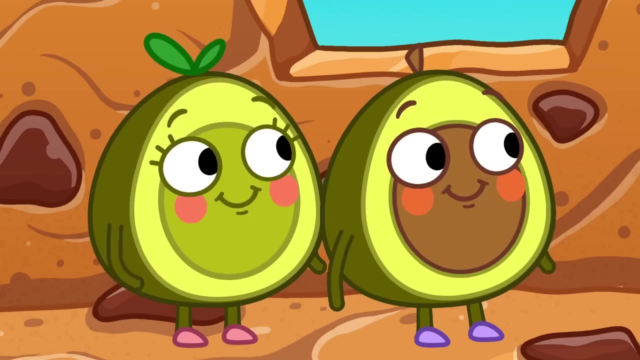 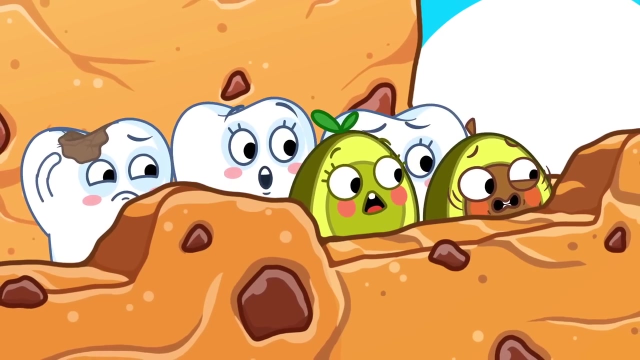 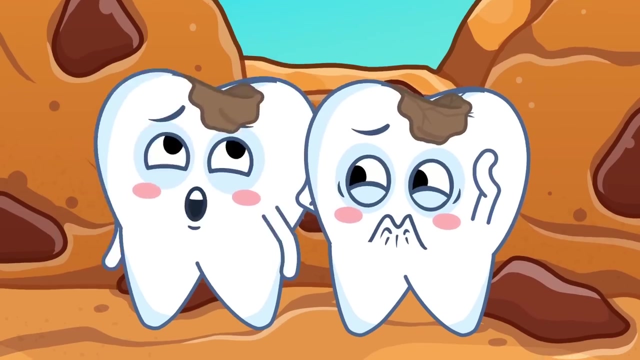 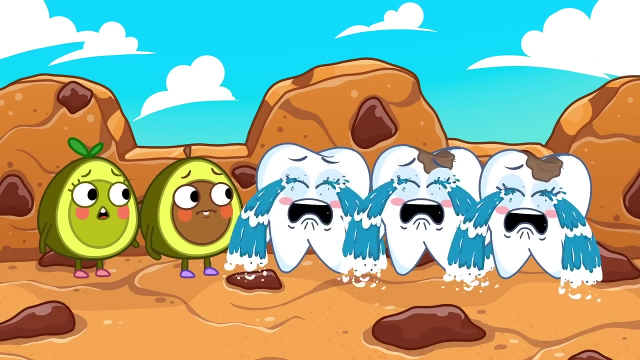 The kids need help. Pit and Penny are safe for now. Thank you, Hey. Hey, The germs are throwing candy. Oh no, Sweets are dangerous for teeth. I know what to do: Toothpaste will stop those germs. 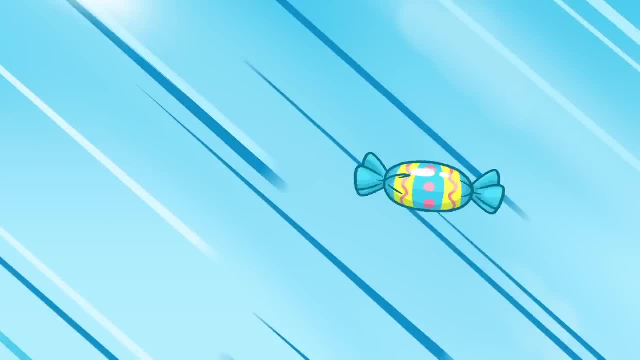 Huh, I would not do that. I'm sure I bet you won't believe me. I swear I didn't. This is going to be normal. I'm not going to die. I'll get better. I'll wait for you. 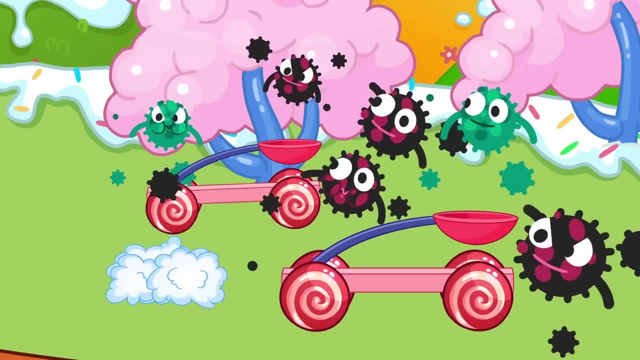 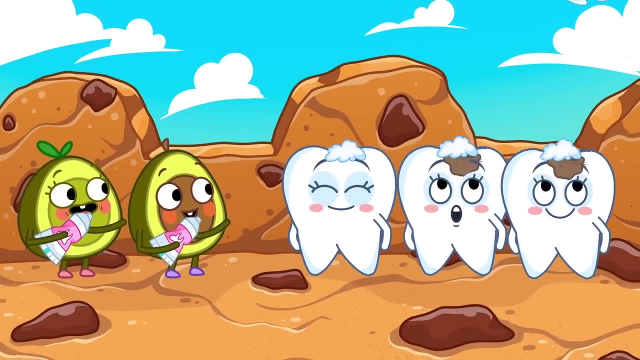 I don't know. I need to be with you. I won't let you there. I knew it. I'll wait for you. I'll wait for you. I promise I'll wait for you. Are you going to eat it? 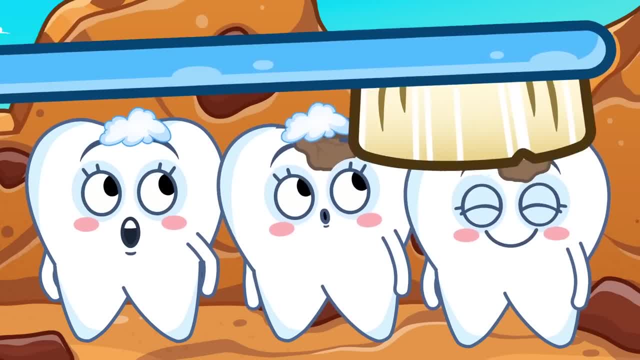 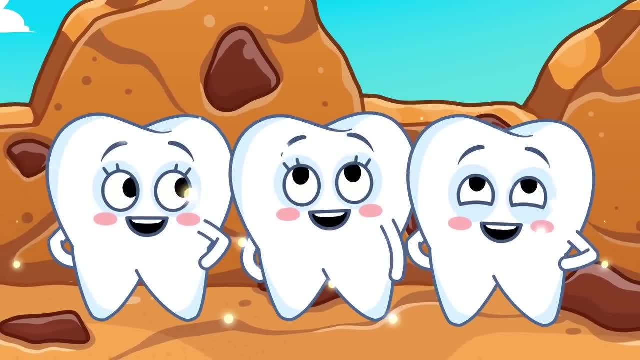 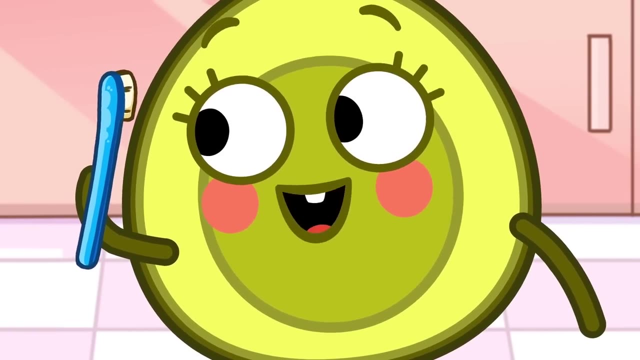 I'm going to make a toast. I need a good taste. Okay, One, Two, Three. I should have more lollipops. One, Two, Three, Two, Two, Four. We need to protect our teeth. You should brush twice a day. 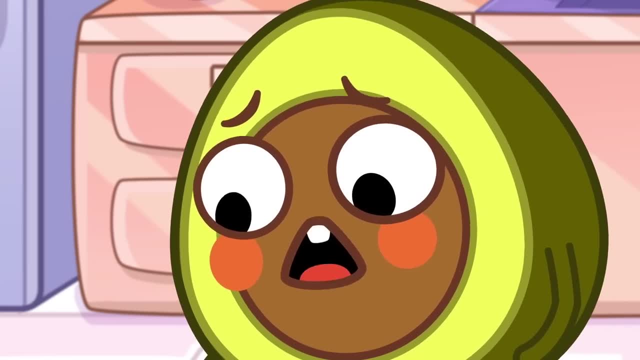 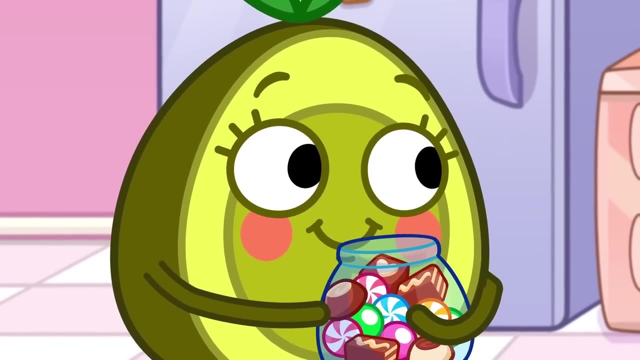 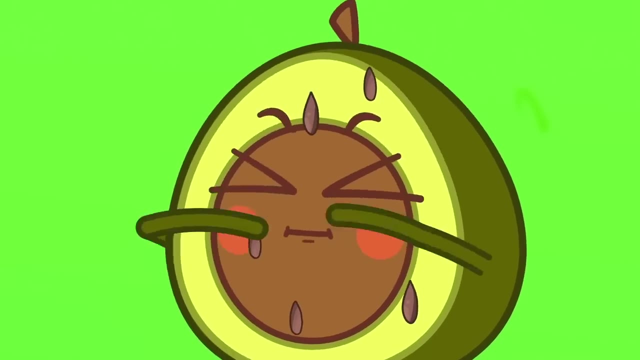 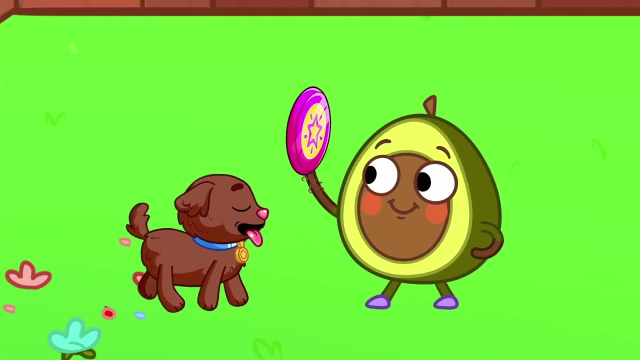 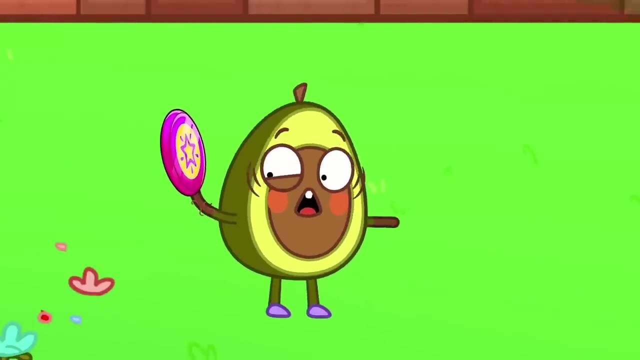 No, Pit. Okay, We can eat just a little bit of sweets. Let's eat another one tomorrow. Good idea: Pit's playing frisbee. Look A puppy. Looks like Pit's getting a little bit dirty. Time to wash your hands. 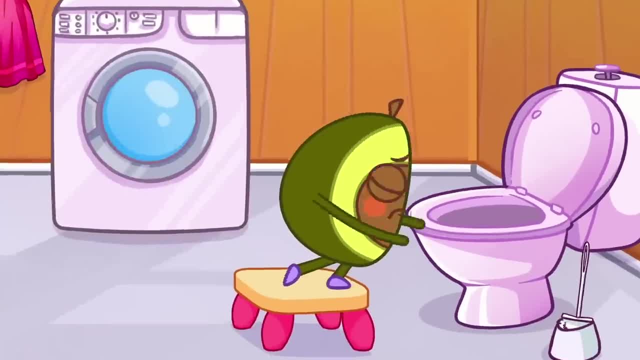 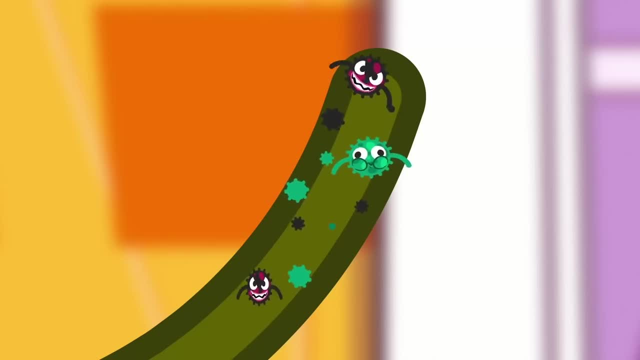 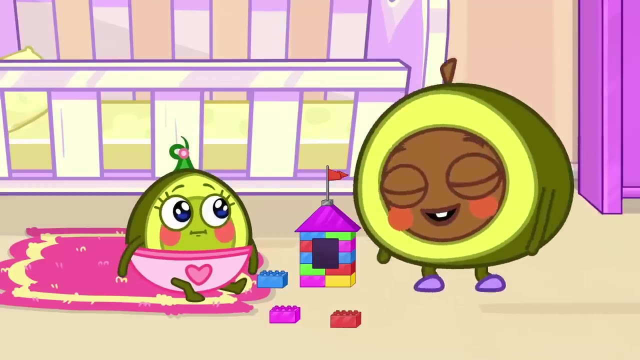 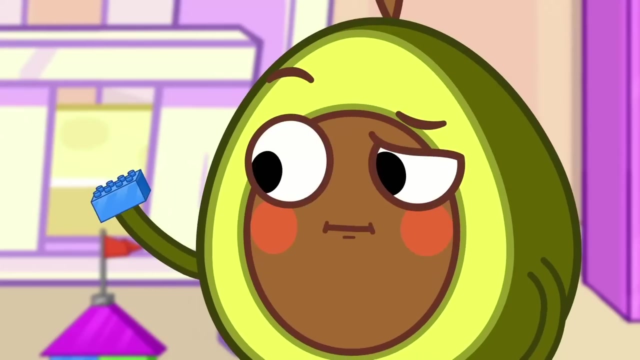 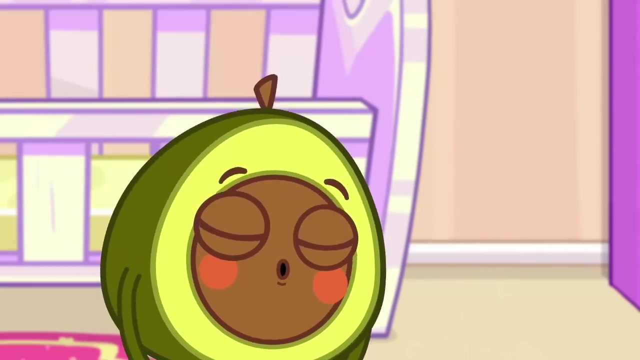 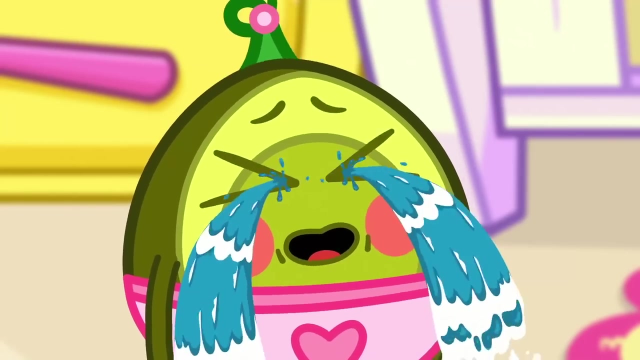 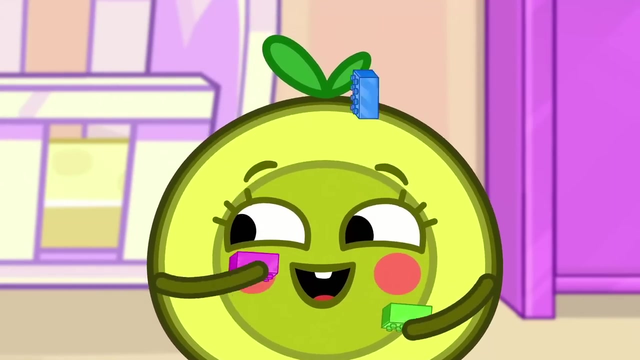 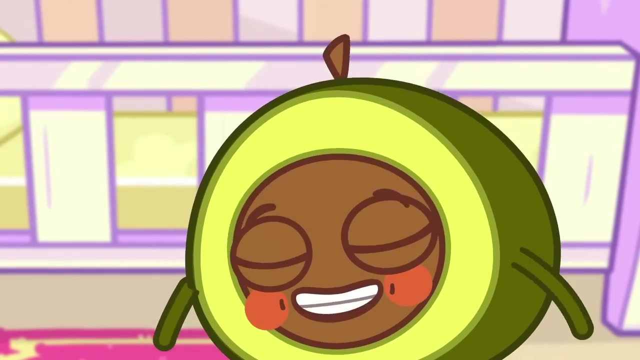 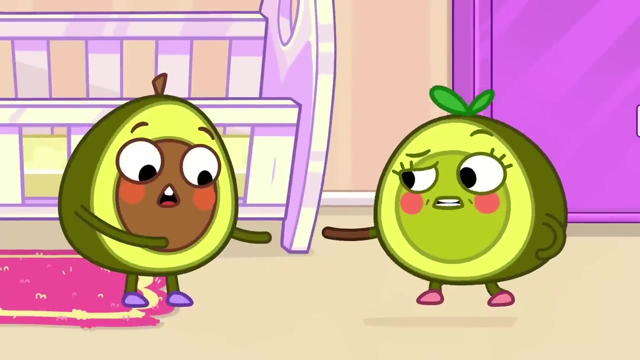 Ew, The soap landed in the toilet. But, Pit, you need to wash your hands. Soap for clean hands. Pit wants to play too Shoot C'mon Penny. Penny can fix this. Your hands are dirty. I've already washed my hands. 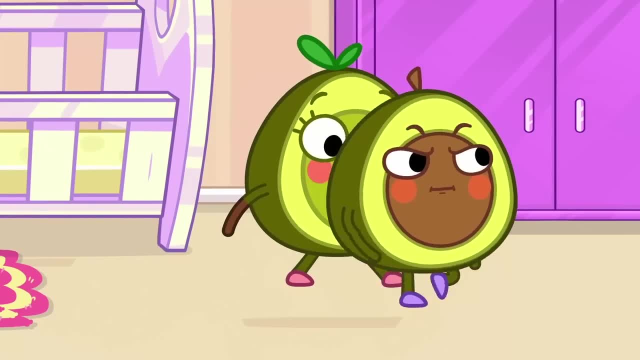 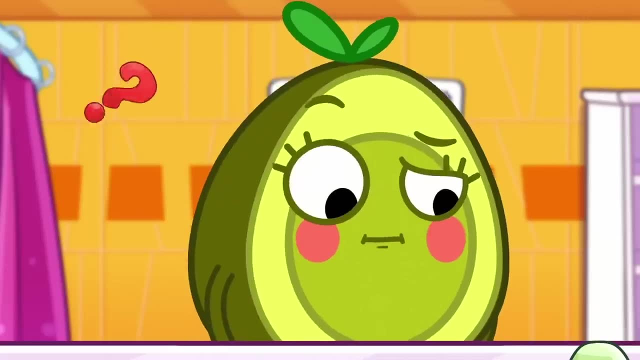 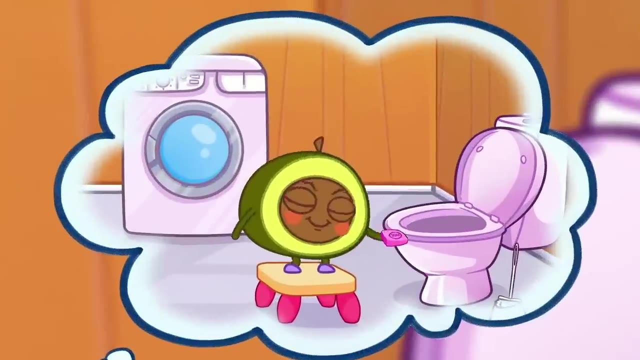 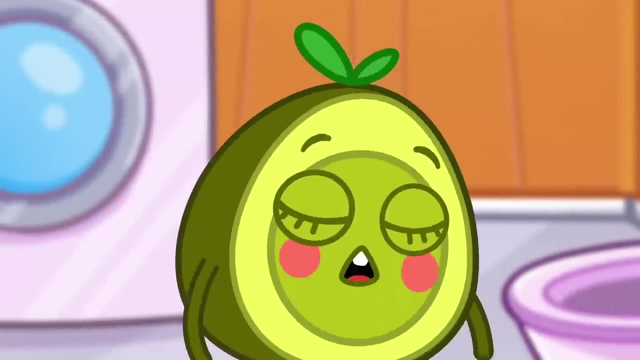 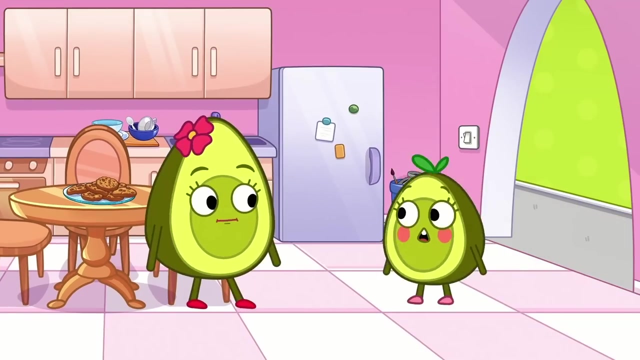 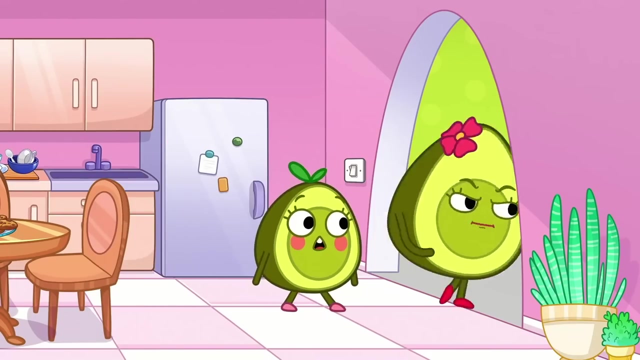 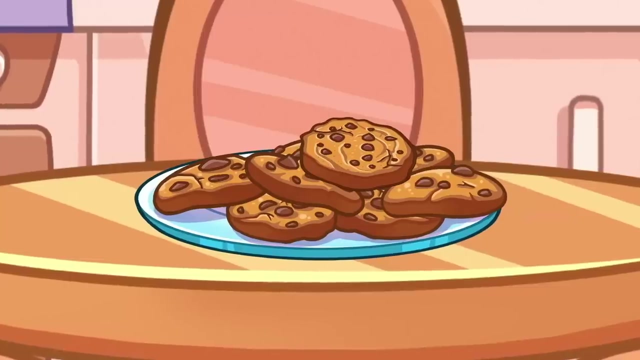 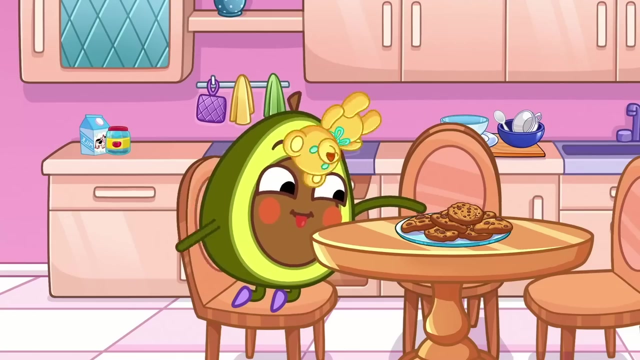 Your hands are dirty. Where's the soap? Penny Pit dropped it in the toilet. Yum, Mommy made cookies. Oh, Pit washed his hands without soap. Pit wants some cookies, But he still has dirty hands. Baby will stop him. 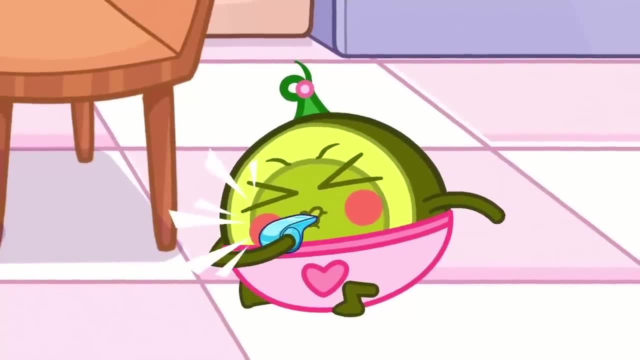 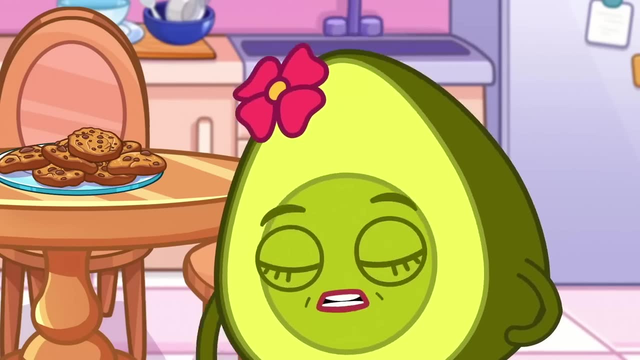 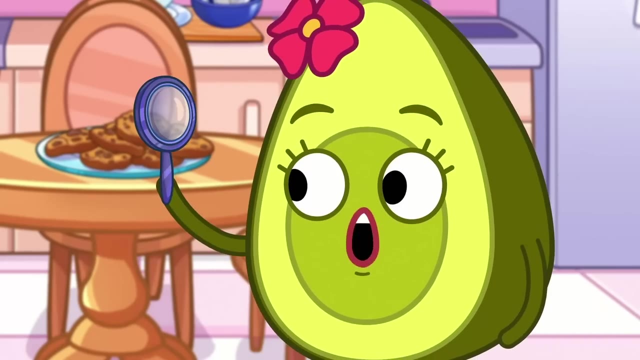 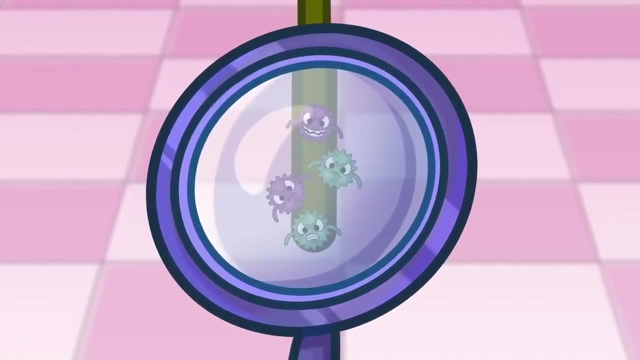 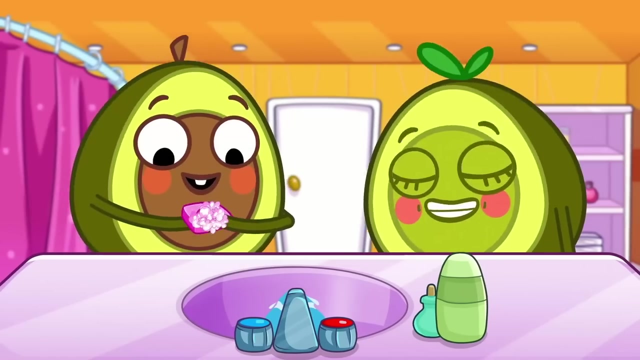 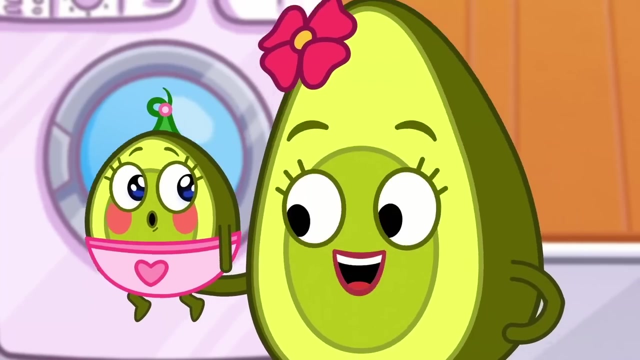 Pit, you can't climb on the table. Always wash your hands with soap. It will protect you from germs. You need to wash again There. The germs are gone. Now it's time for lunch. Pit and Penny can't wait. 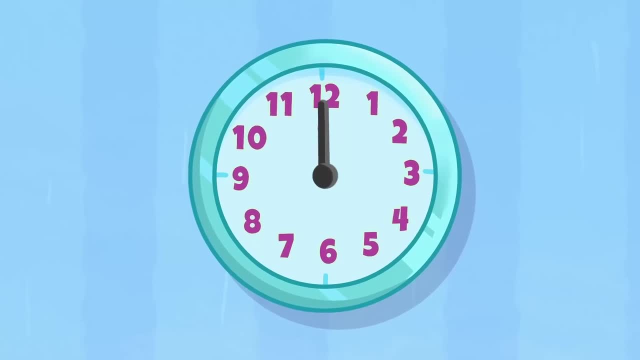 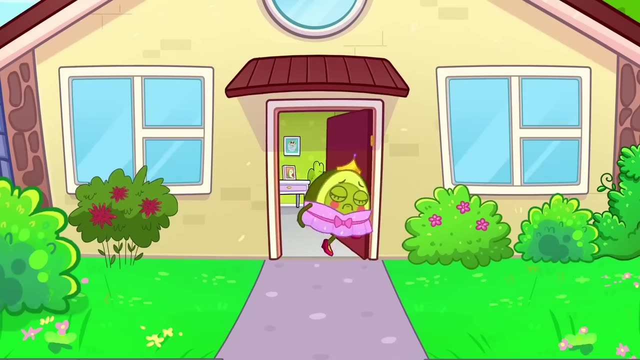 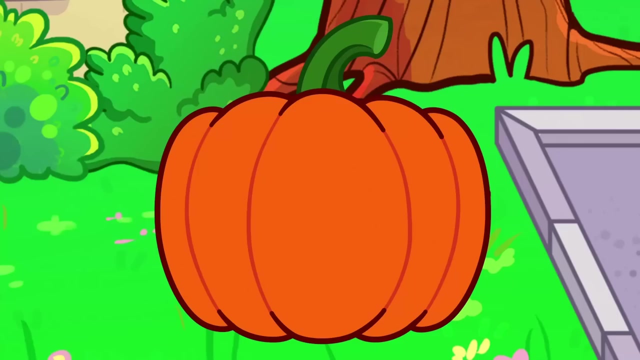 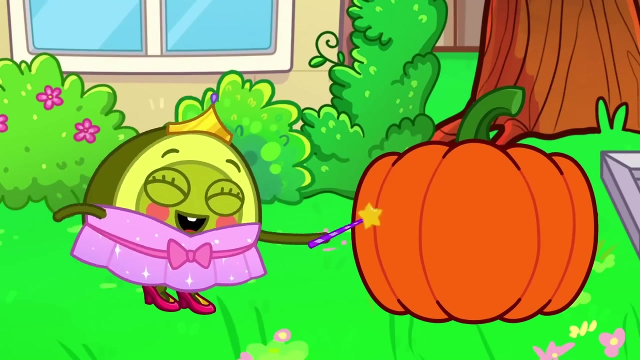 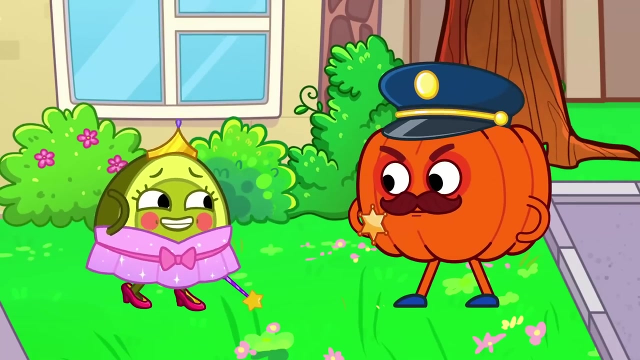 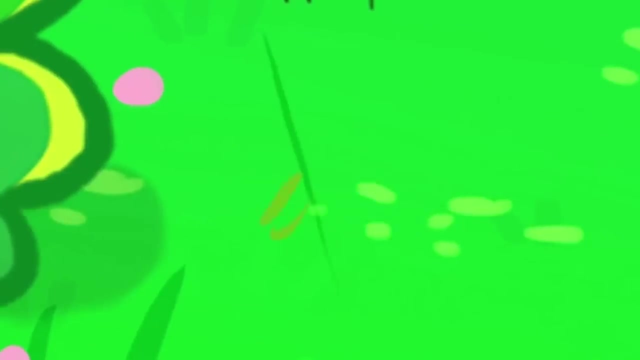 Penny is pretending to be a princess today. I'm late for the ball. You better hurry. And where is my carriage? You can use that pumpkin Abracadabra. Oops, It's Officer. Pumpkin Penny lost her shoe. Oh, Someone took it. 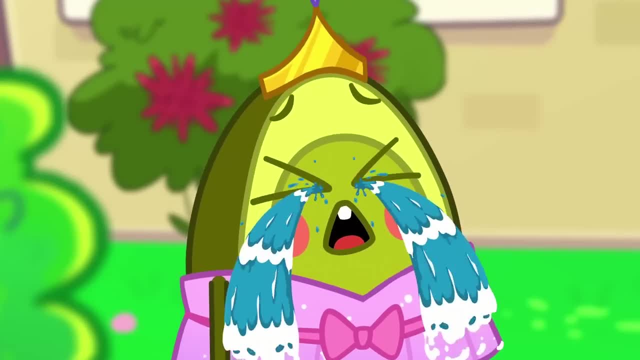 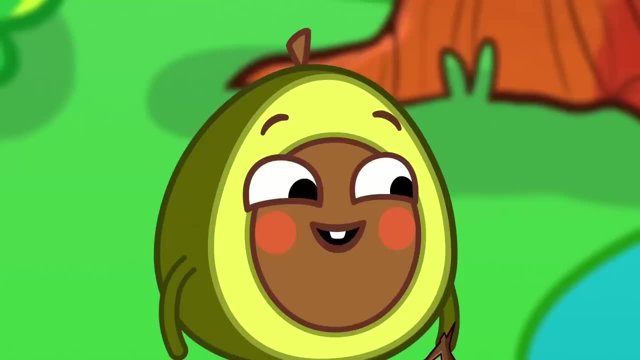 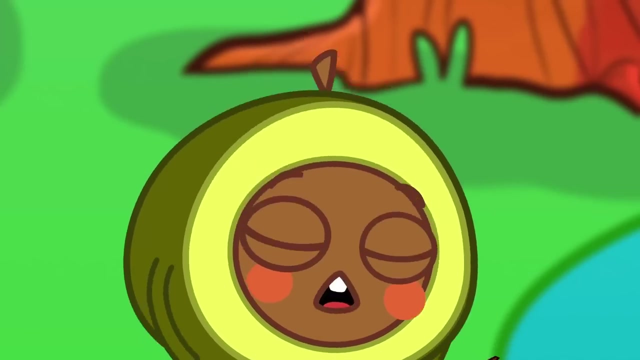 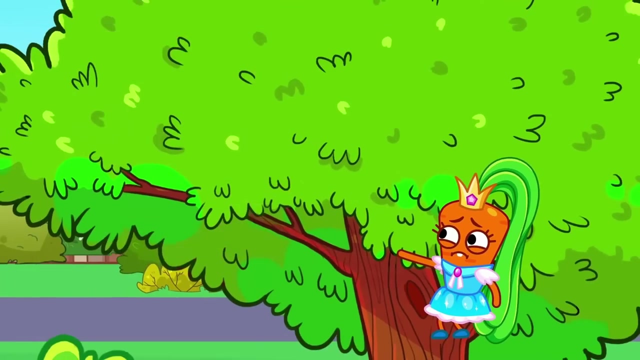 Aw, Robinson took it. Pit's using the shoe as a boat. Pit's using the shoe as a boat. Hmm, Ah, Ah Ah. Carrot's afraid of dragons. Oh ow, Oh, Ah, Ah, Ah Ah. 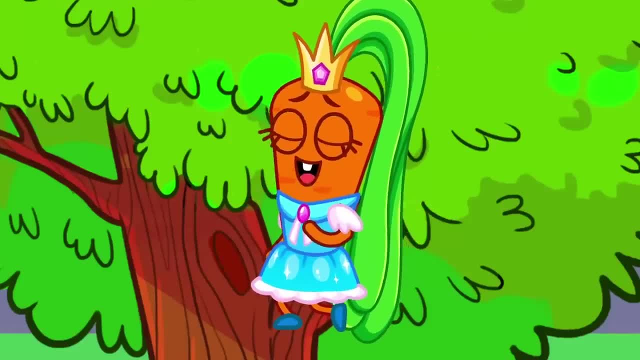 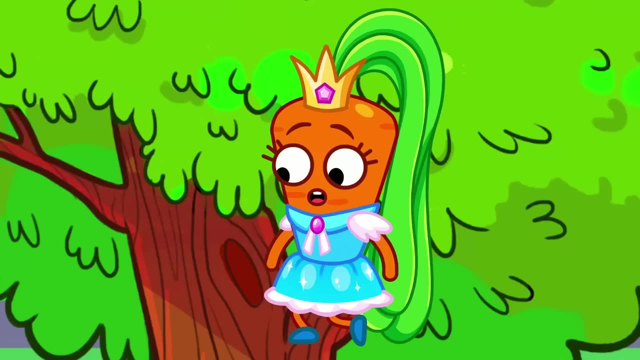 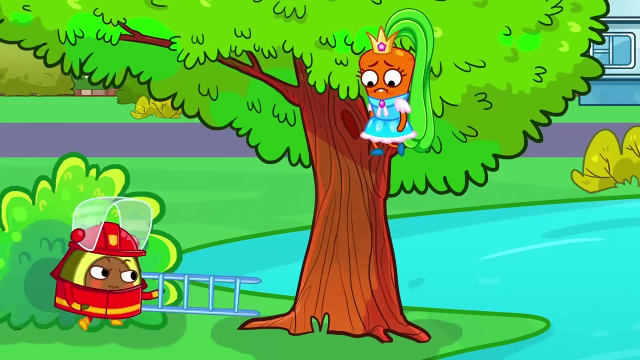 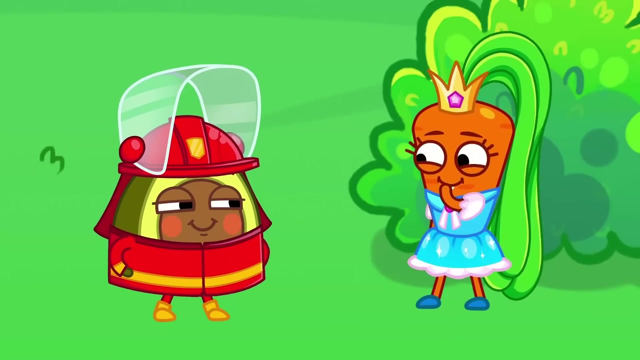 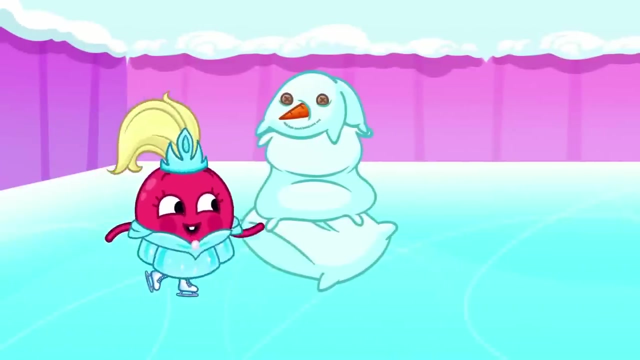 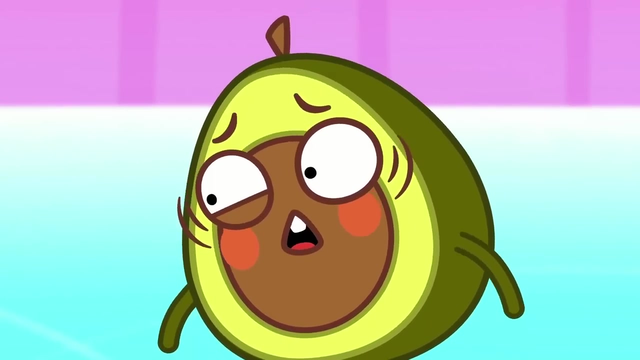 Ah, Ah, Ah. Good prince, save me please. Pit doesn't want to be a prince, He'll be a firefighter instead. He's here to save you, Carrot, But no kisses please, Pit. Cherry needs you. 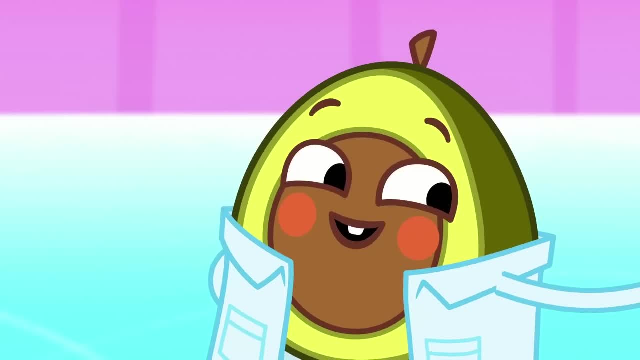 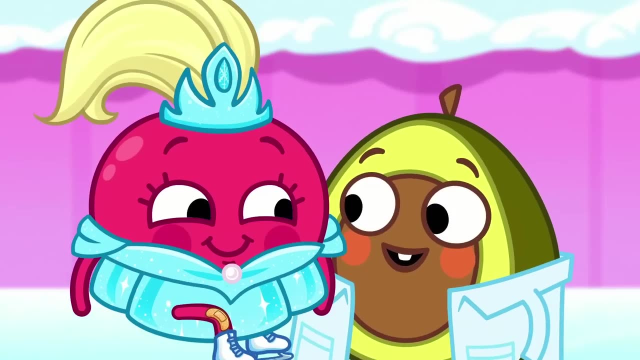 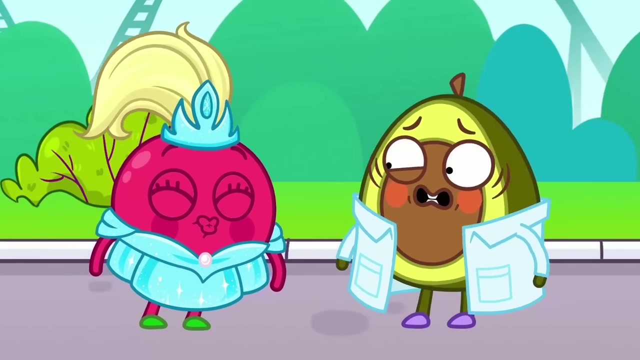 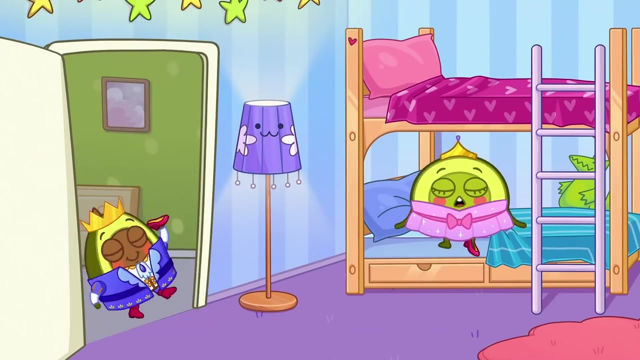 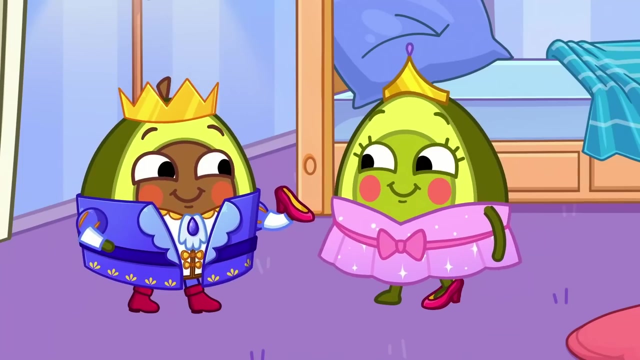 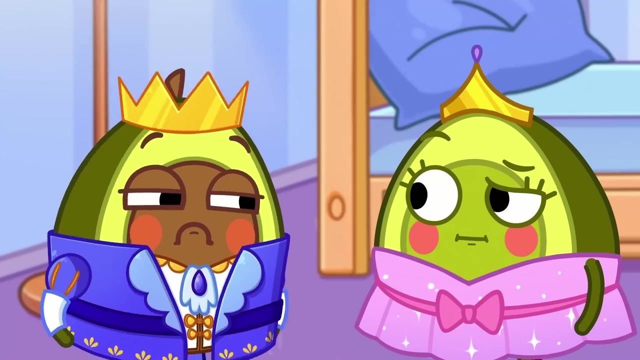 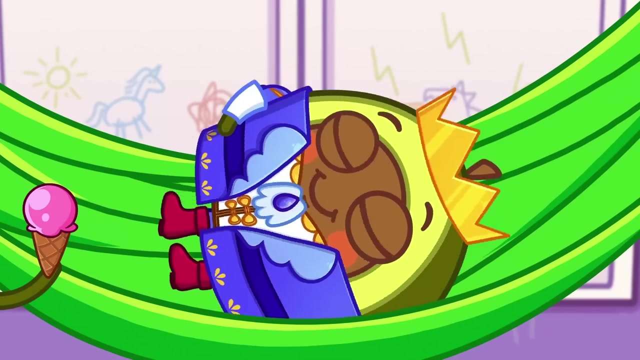 Pit will be a doctor. He'll help Cherry feel better. She thinks Pit is a prince, But no kisses please. Pit has your shoe, Penny, Now. Pit's tired from helping all the princes, But they want to thank him for all his hard work. 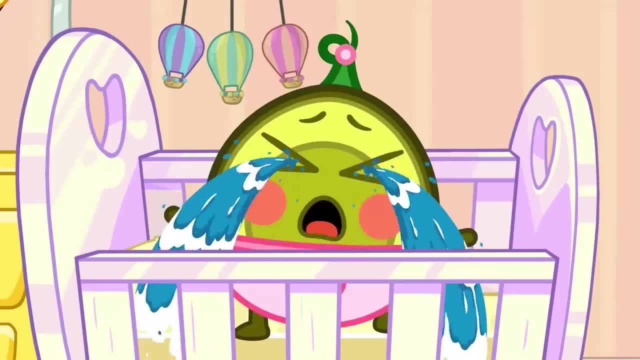 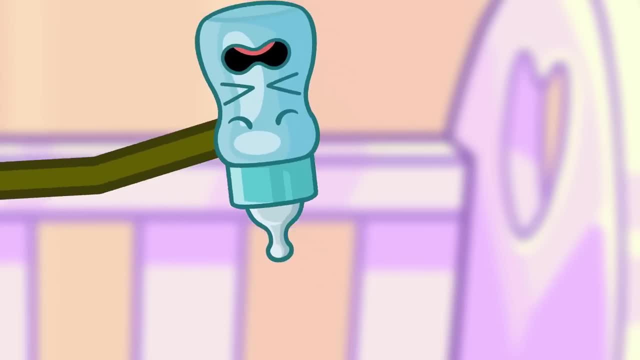 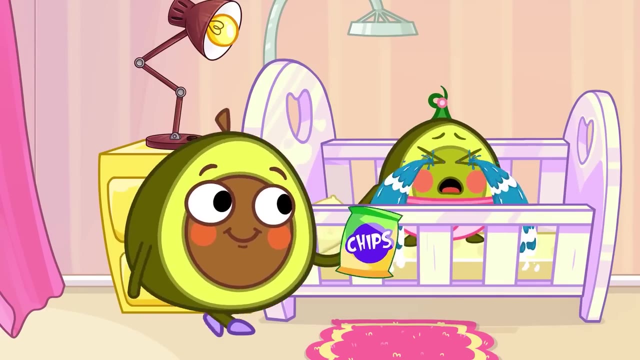 Nighty-night Prince Pit Hurry, baby's hungry. Oh no, there's no formula left. He has no idea what he's doing. Without the formula, Pit can't move. Maybe I'm just a little more careful. Ah, I'm just a little too old to do this. 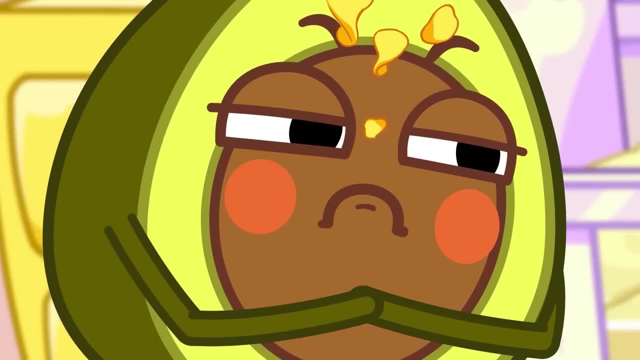 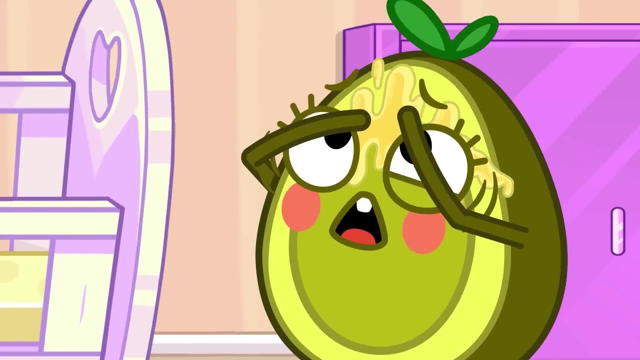 Just do it, baby, You can have one. No, no, no, no. I want another banana, But it's too big for me. I wanna eat it. No, no, no, no. I have to lay it on the floor and wait for him. 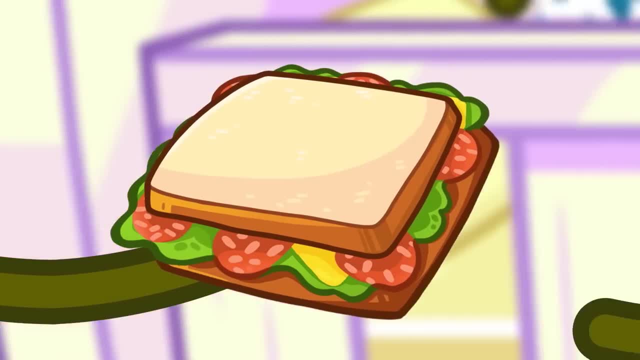 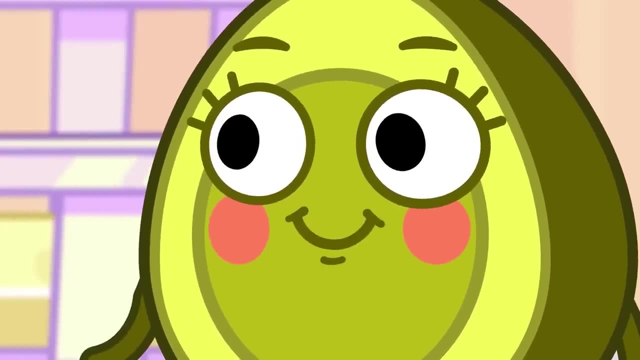 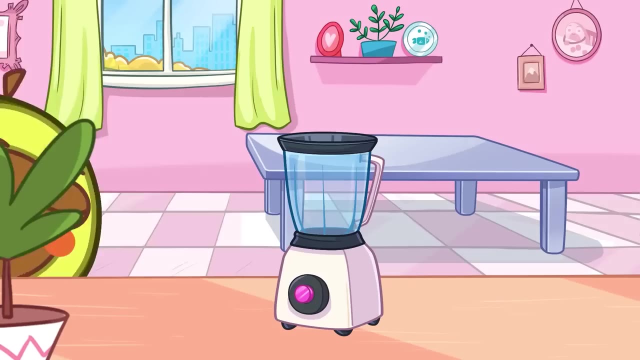 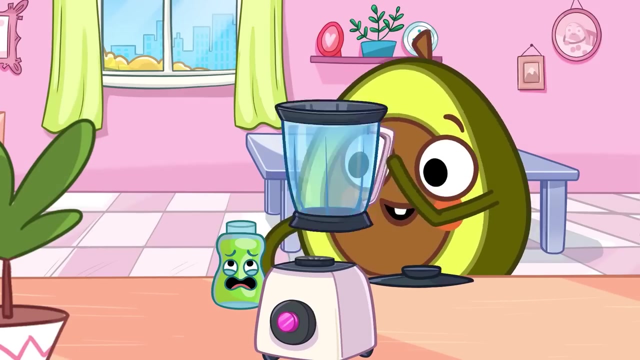 You're a little too of a girl. You can't stop me. Let me help you, I can do it. Baby can't chew because she doesn't have teeth yet. Pit has an idea: He'll make a sandwich milkshake. It looks awful. 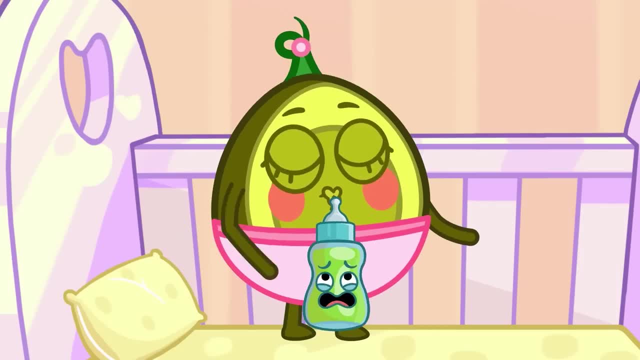 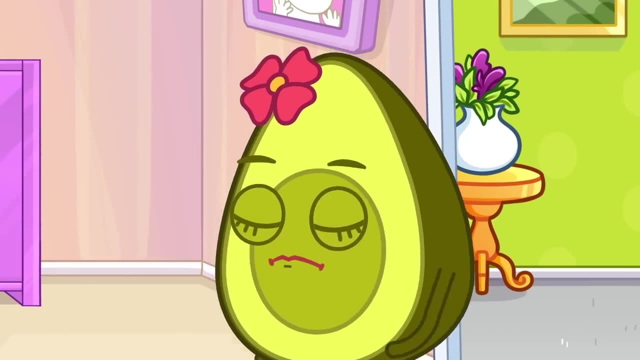 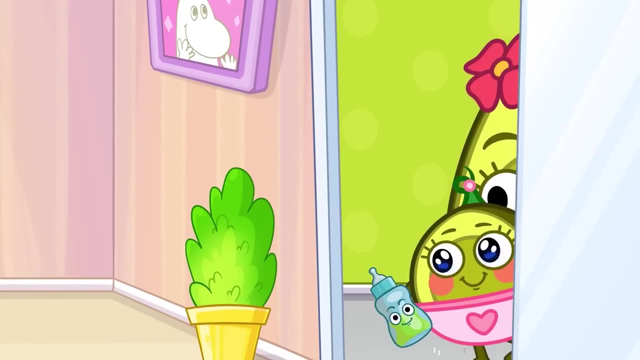 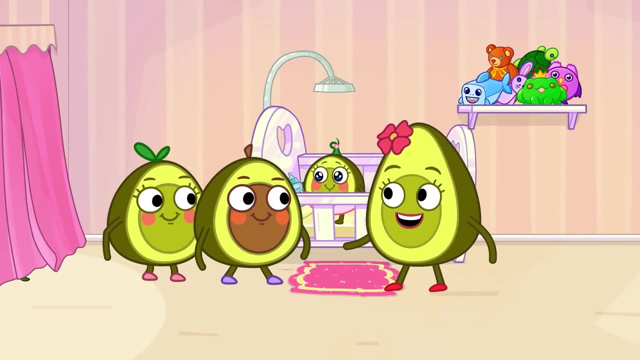 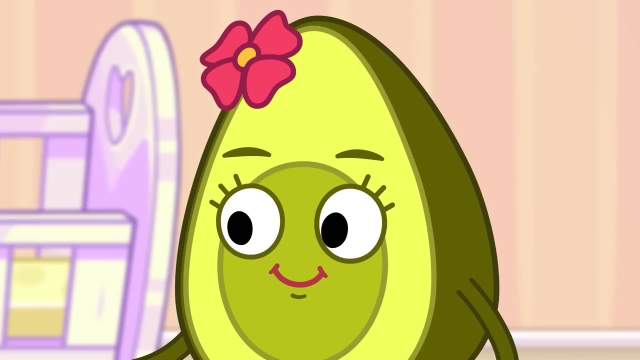 And it gave Baby the poopsies. Don't worry, Mommy will change her Now she's nice and clean. Babies shouldn't be fed regular food. What do you mean, Mommy? You need to prepare formula for the baby. 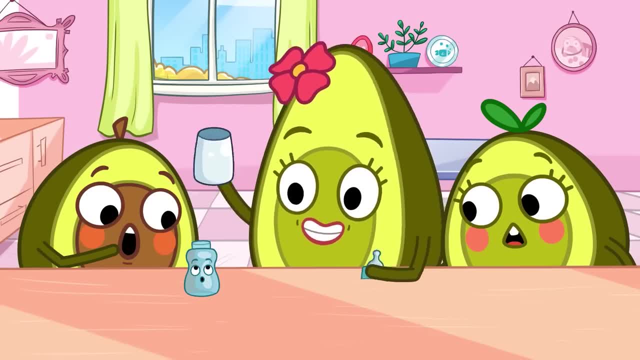 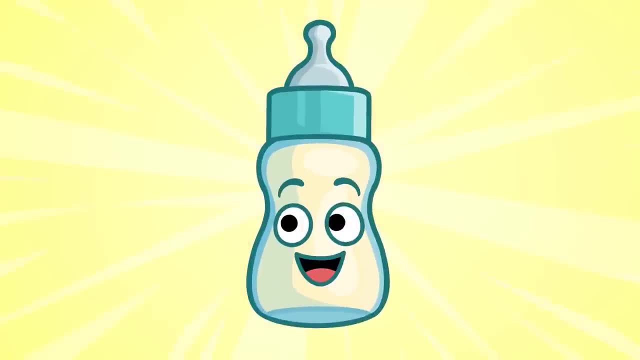 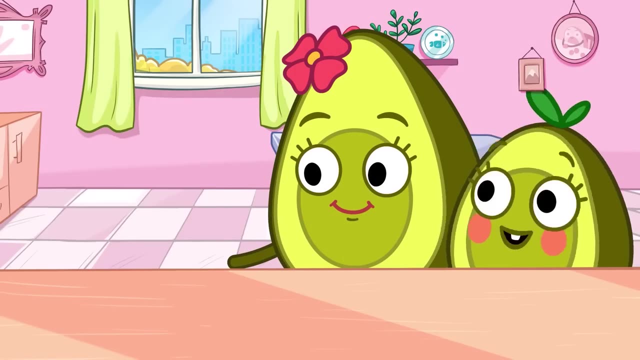 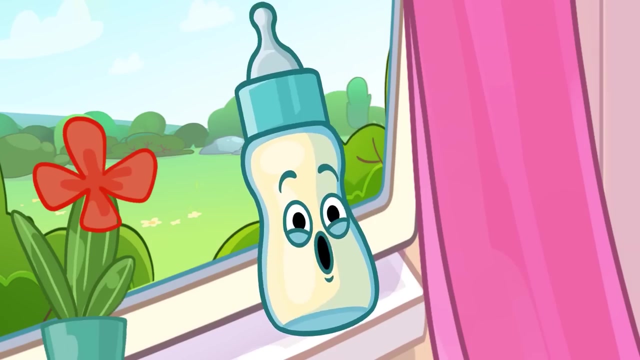 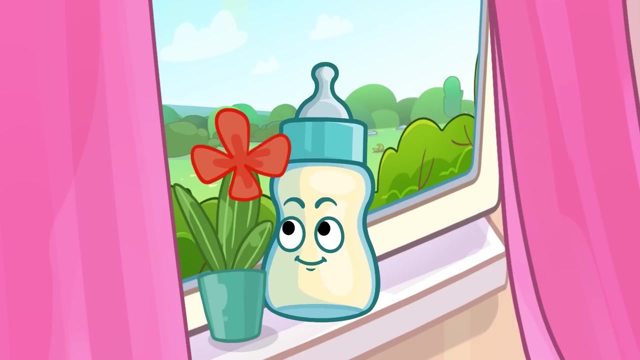 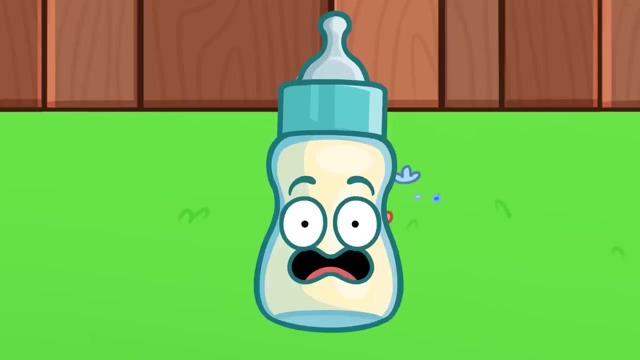 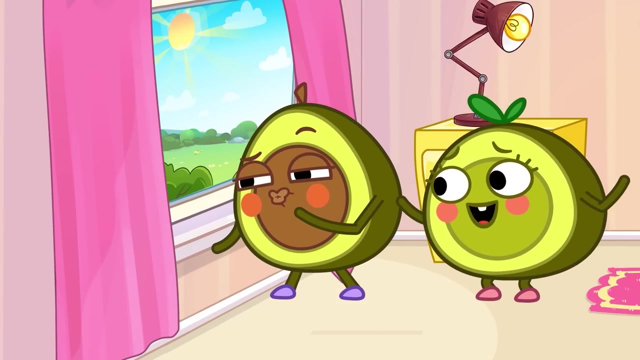 First you need a baby bottle. Then you mix the formula with some water. This is food for babies. Now you can feed the baby. Whoa, It's okay. Pit, The bottle is by the window. Achoo. What do we do now? 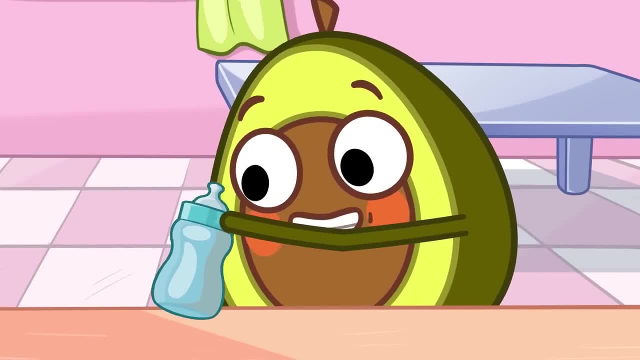 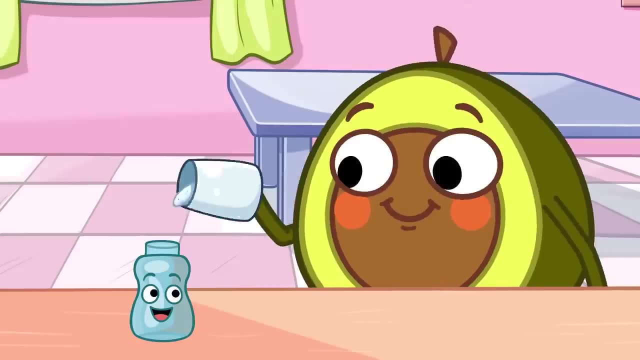 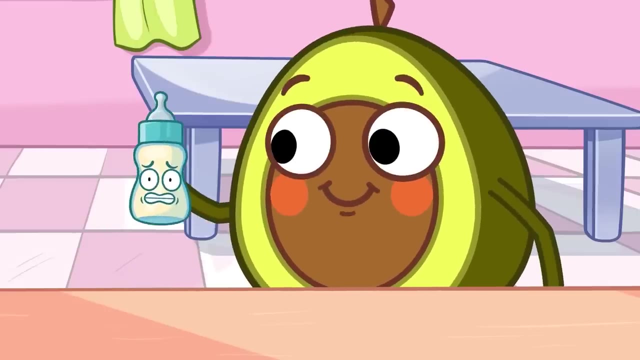 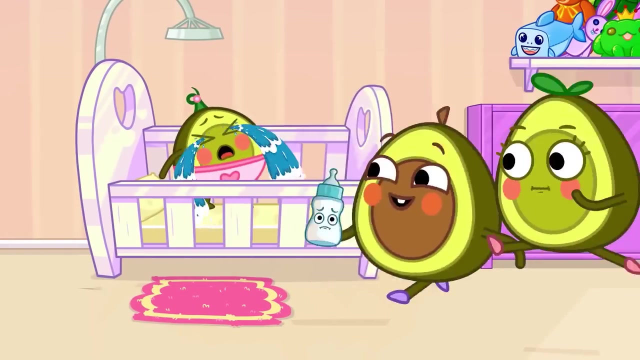 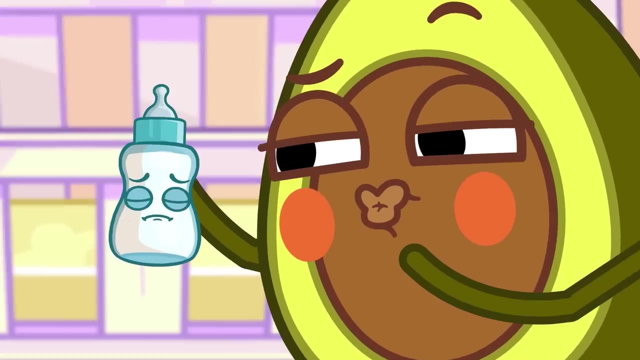 We will prepare the formula ourselves. I hope you know what you're doing. Pit, Okay, Now add some formula. What about the water? Pit? That doesn't seem right. It won't come out of the bottle. Whoa, Whoa. 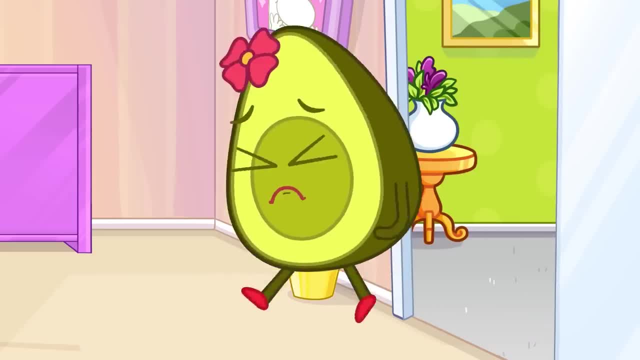 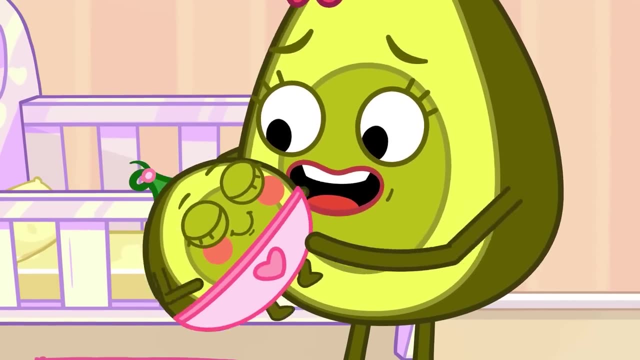 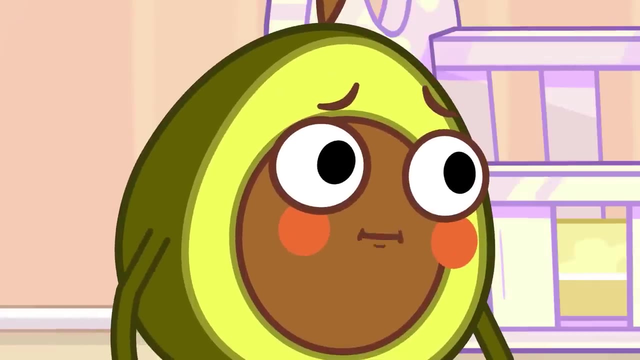 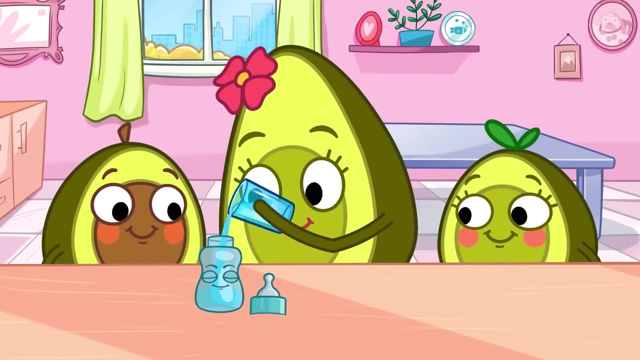 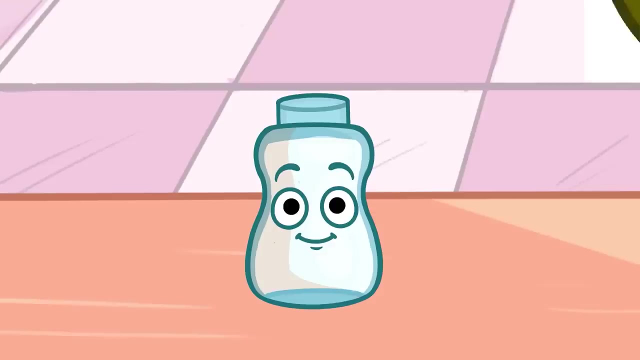 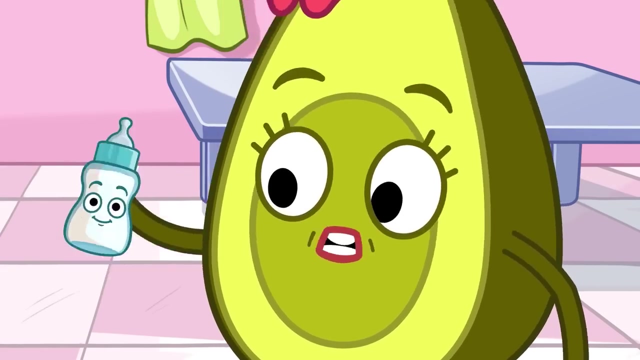 Whoa, Whoa, Whoa, Whoa. We wanted to make our own formula for a baby. Never be afraid to ask for help. You need to remember the water next time. Then add a little bit of formula. You need to put three tablespoons of the formula. 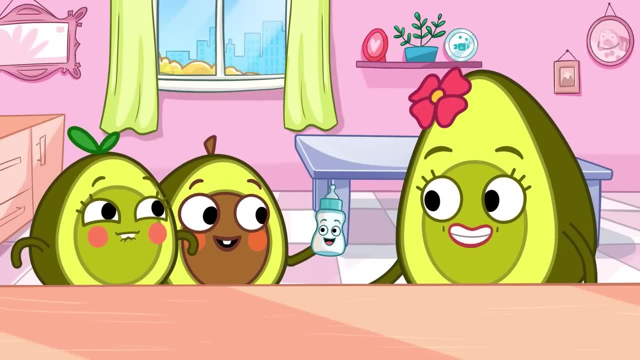 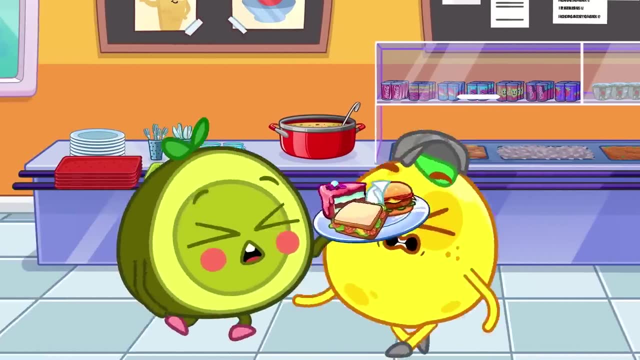 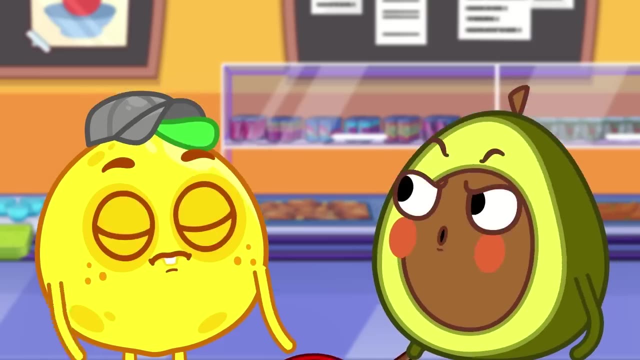 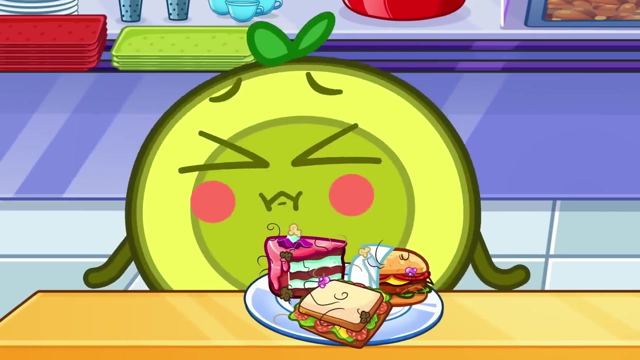 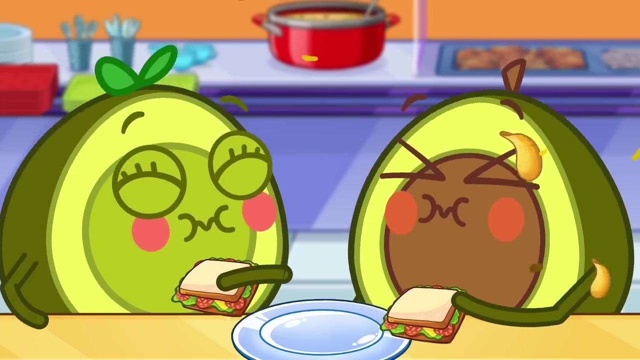 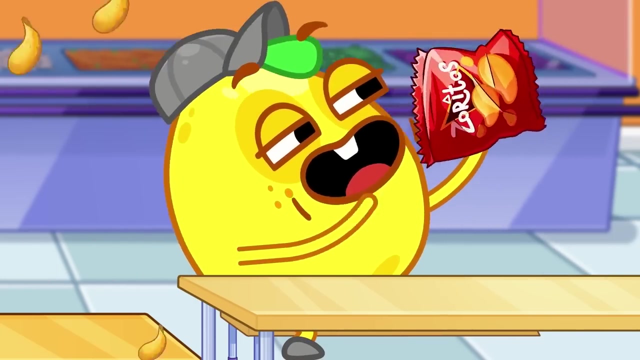 And shake. Now we can feed babies Ketchup. Be careful, little lemon, You hurt Penny. You shouldn't run Now. Penny's lunch is ruined, But Pit will share his lunch. Little Lemon is making a mess. No, no, no. 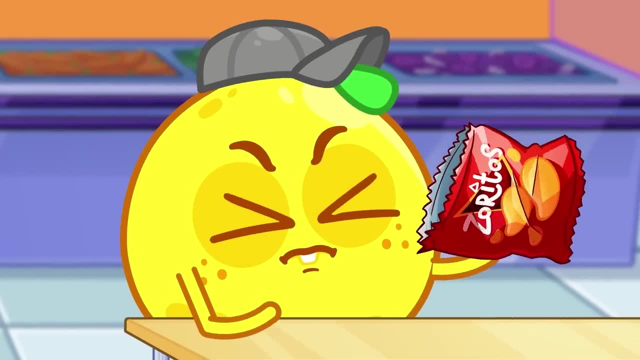 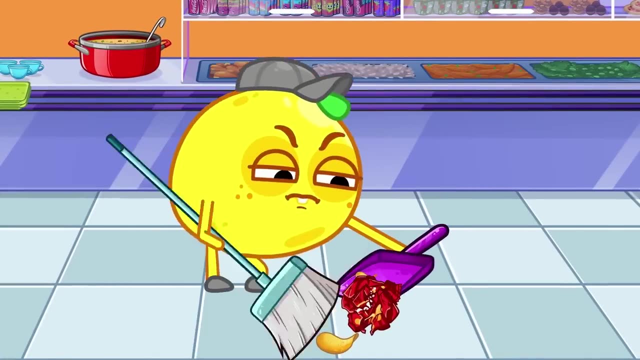 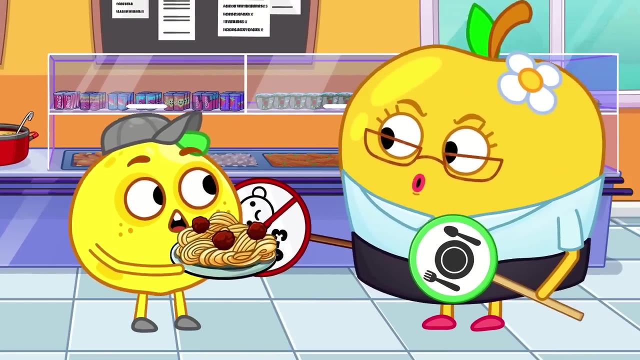 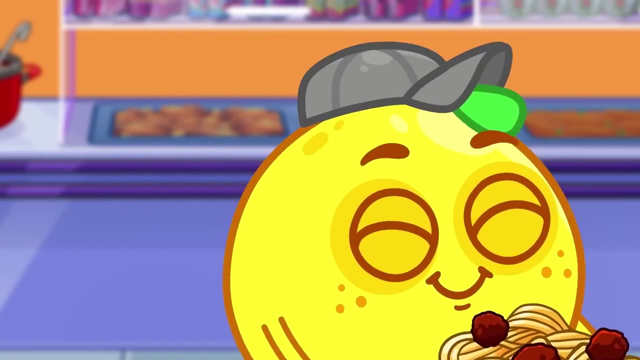 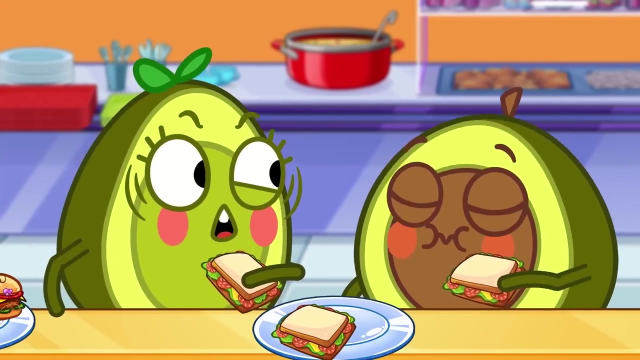 No trash Little Lemon will have to clean it up. Duh, This cool cafeteria is for eating, not for playing. What's Little Lemon up to Ahem? Hey, What's up, What's up, What's up. 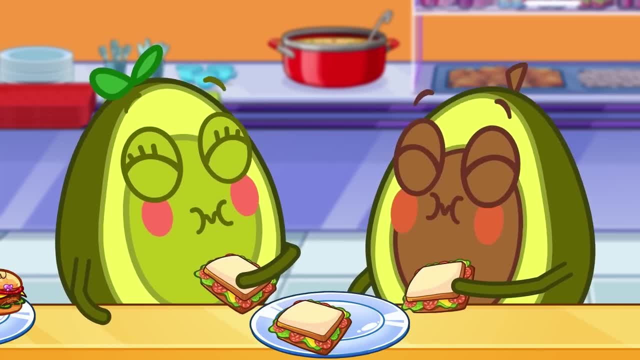 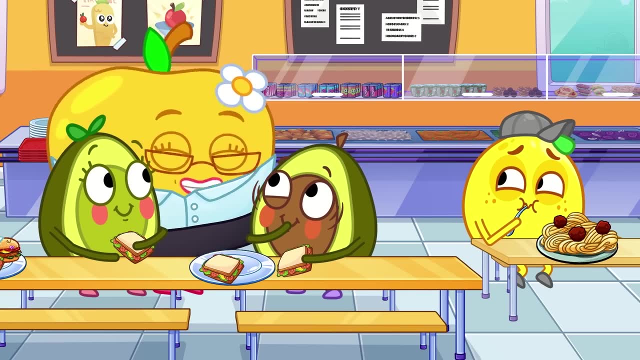 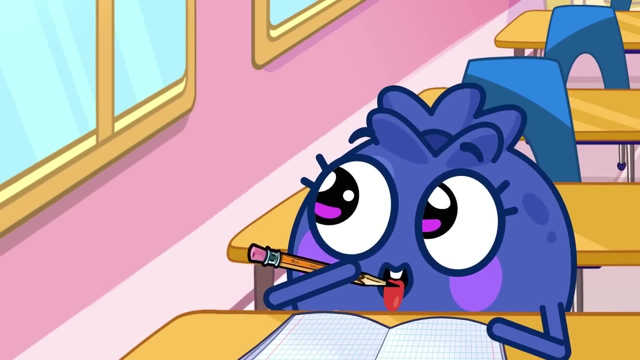 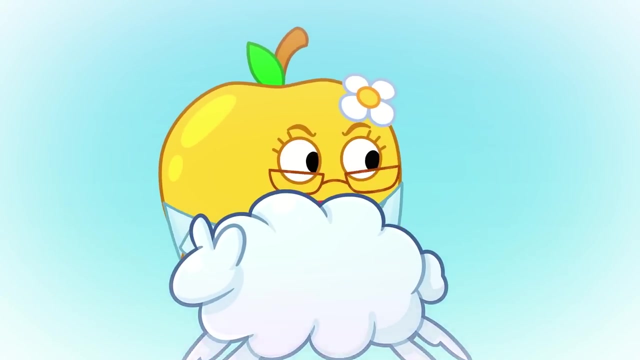 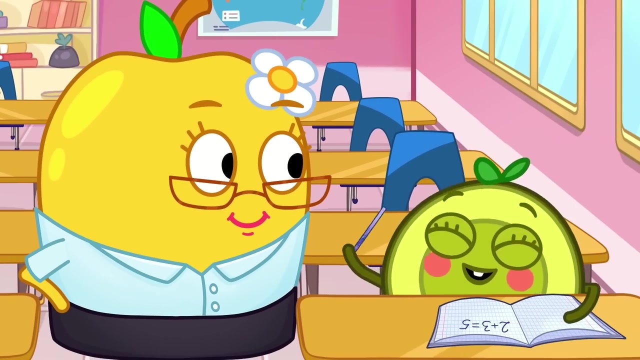 See if I can get you some good food. It isn't forbidden Because everybody burps Blueberry's busy daydreaming. Miss Apple doesn't look happy. Let's check it. Uh-oh, Two plus three equals five Great. 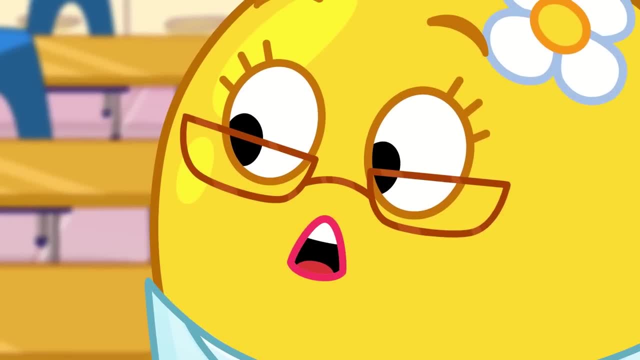 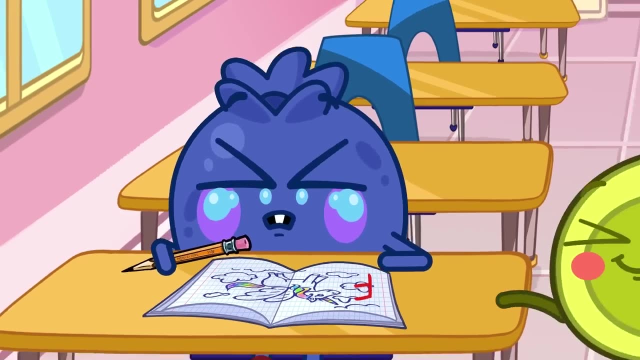 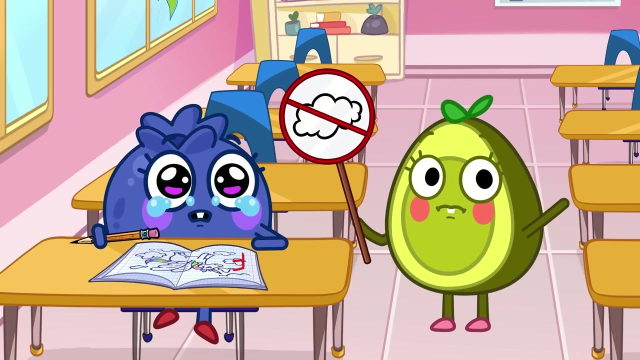 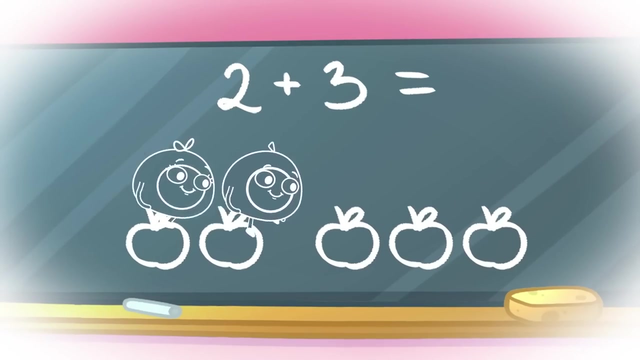 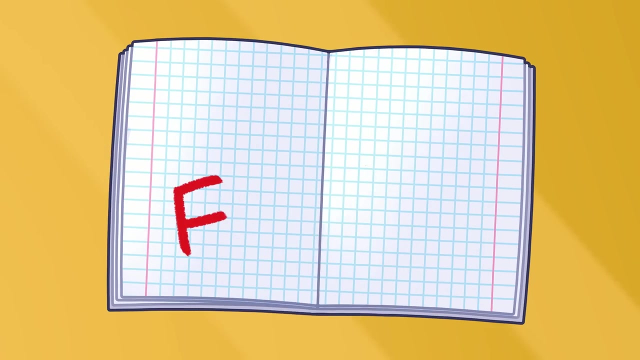 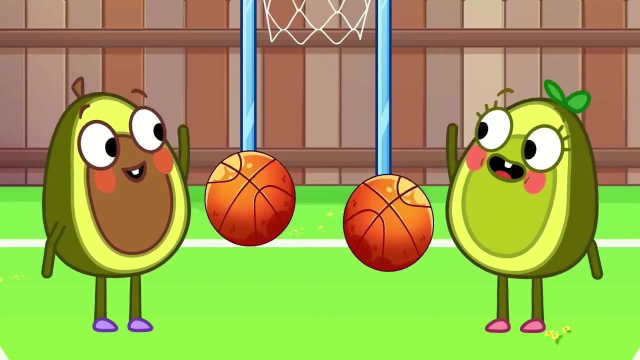 Blueberry drew a picture. instead of doing her math, You should listen to your teacher. Penny will help. One, two, three, four, five. You did it, Blueberry. Great job, girls. It's basketball time, He-he-he. 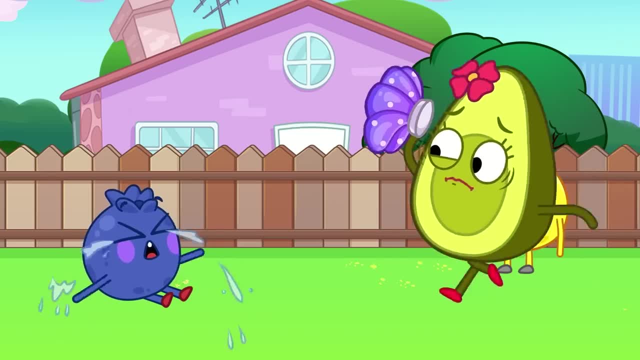 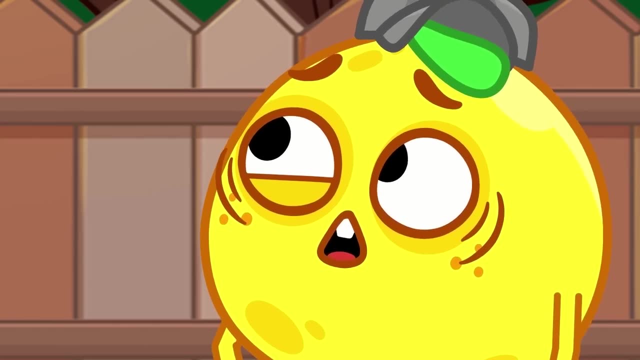 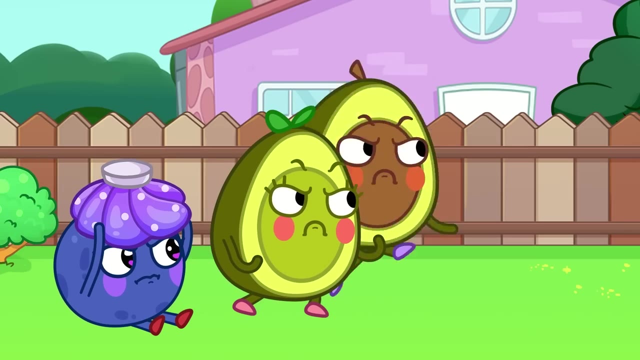 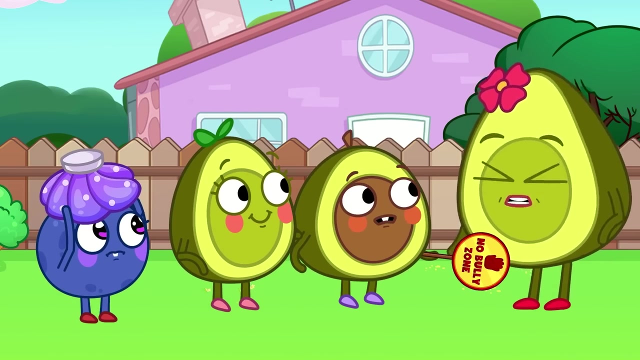 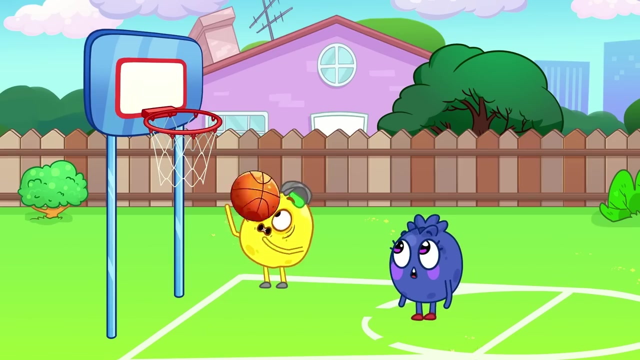 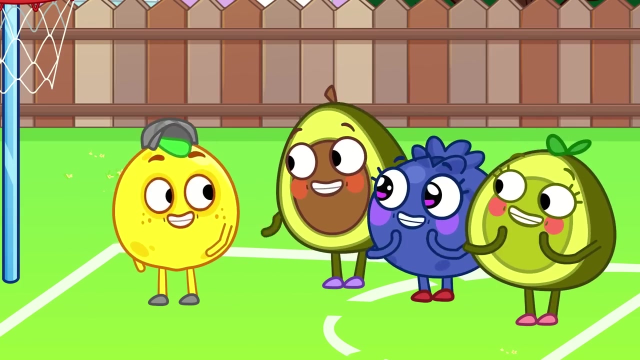 What happened? Little Lemon hurt Blueberry with the ball. You can't hurt your classmates. Don't be a bully. Hey, You have to follow the school rules. I'm sorry, See, It's better when we all get along. The kids are playing hide-and-seek. 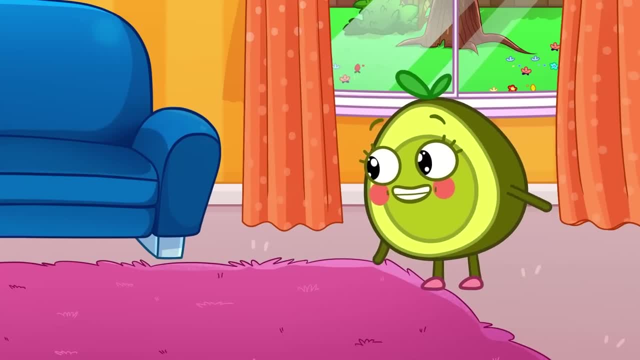 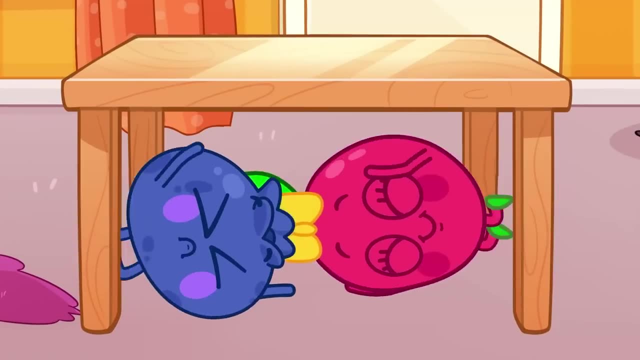 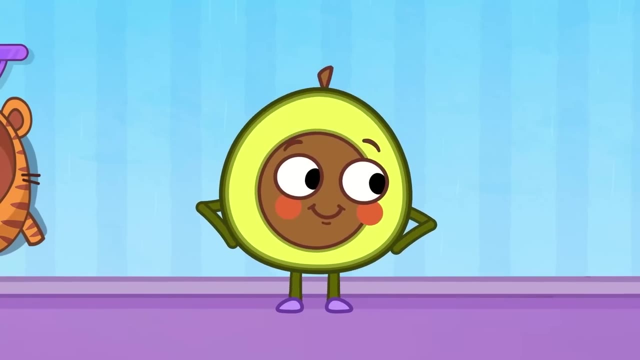 Where should Penny hide? Not under there, Penny, So it's better if I hide under the crossita. I'm sorry, Linda, No Ready, No Ready. Let's stay like this. The three of you are going to hide here. 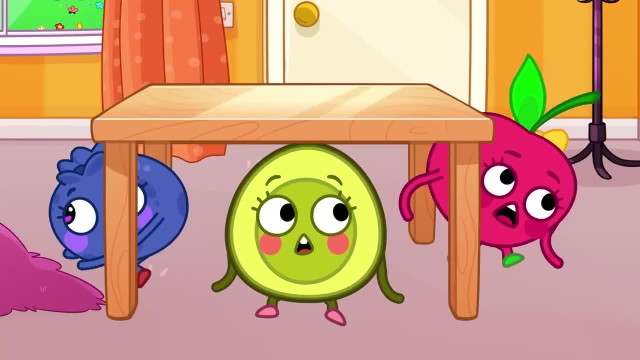 Plănkin and Pinkie: High five. anyone Pl 0910 has finished Down with zeigt Carey, because to play You've got to play with me. How about we start with me? Who wants to play first? Miss Piggy? 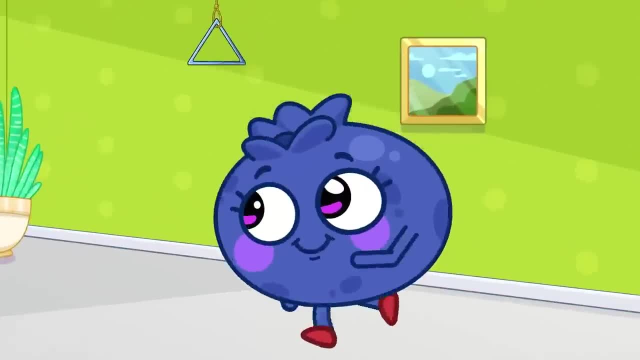 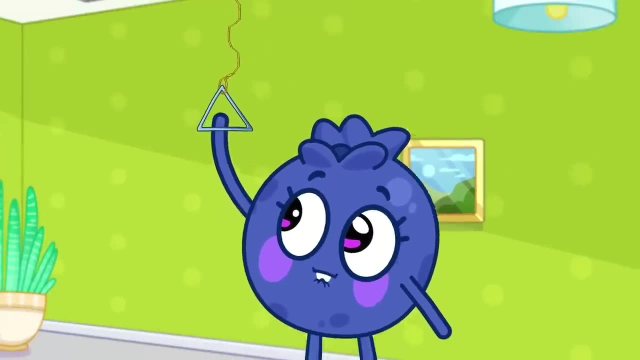 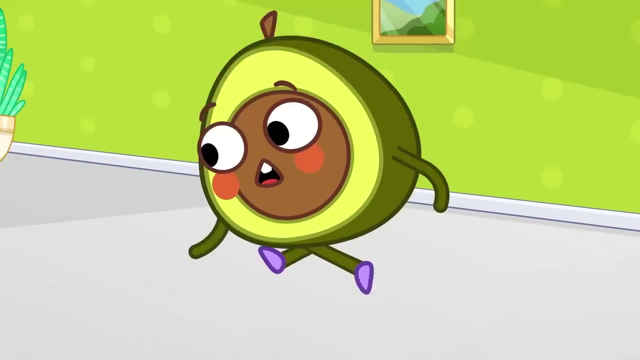 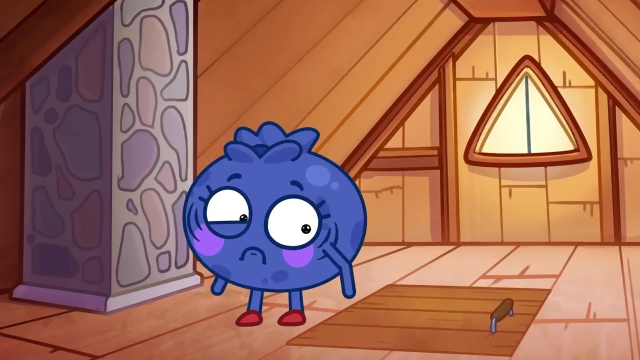 Do you think you're악? Nope, Prim Pichu, How did you do? You three need a better hiding spot. Blueberry wants to hide in the attic. Hit, can't find anyone. Blueberry's stuck in the attic. 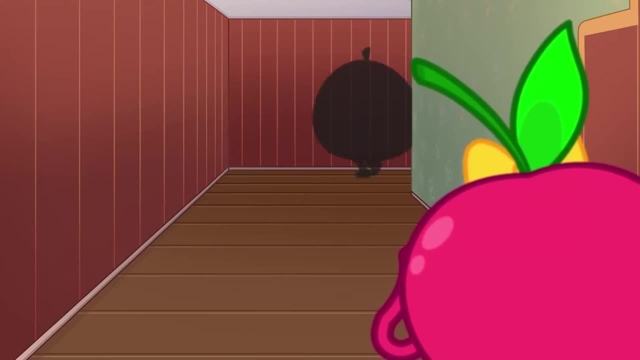 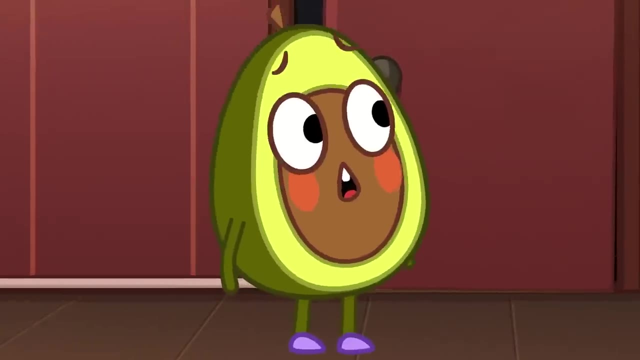 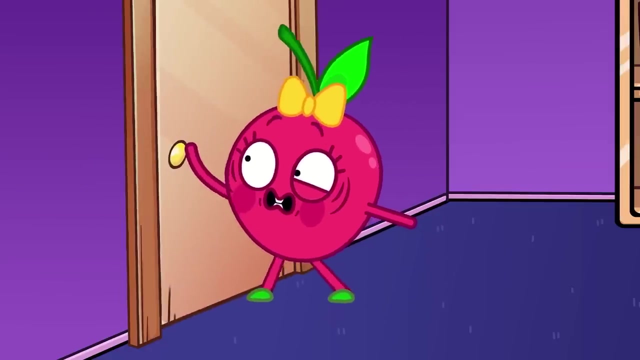 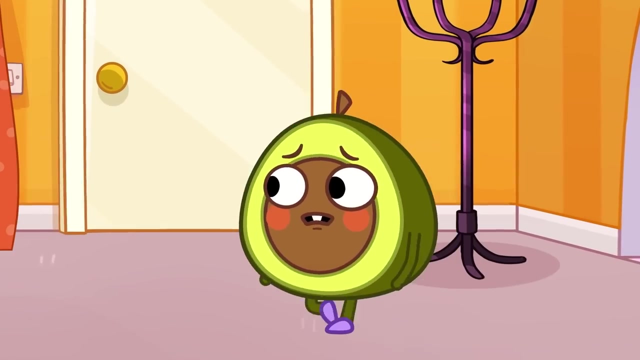 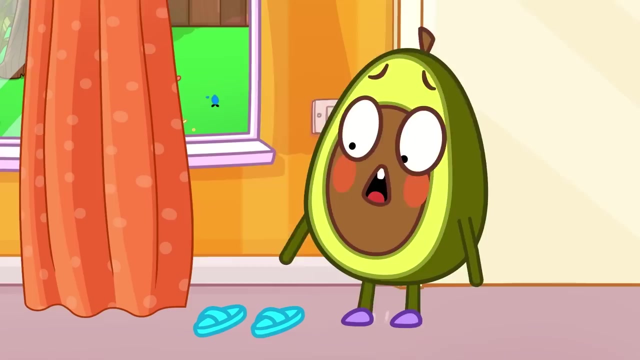 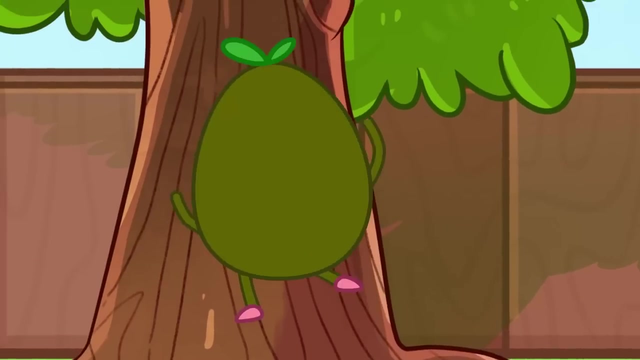 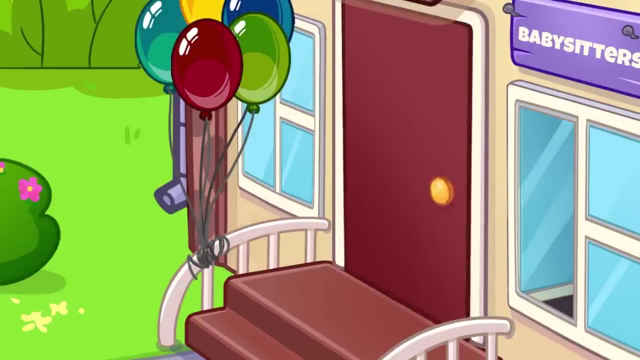 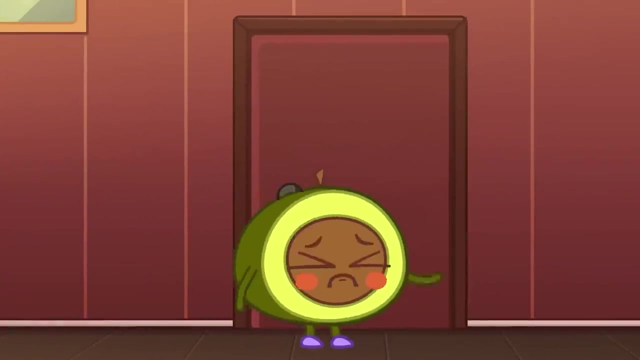 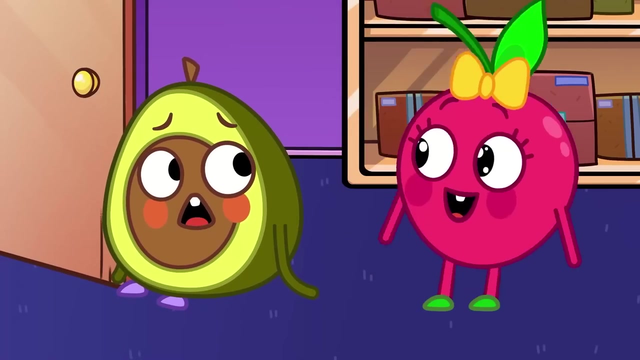 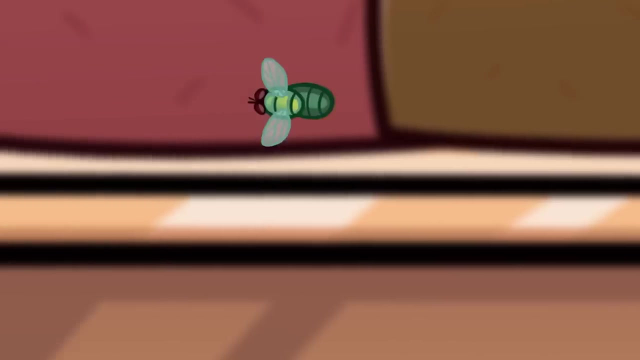 Quick Cherry hide. Now Cherry's stuck in the closet Hit. is that Penny's hiding spot? It was a trick. Penny's hiding outside, Penny's stuck in the tree. You found Cherry Hit, Thank you, Oh no, an annoying fly. 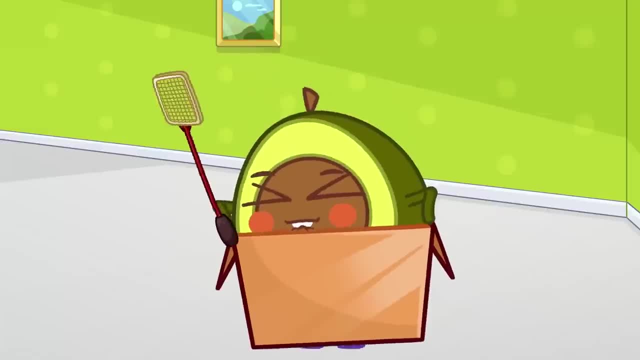 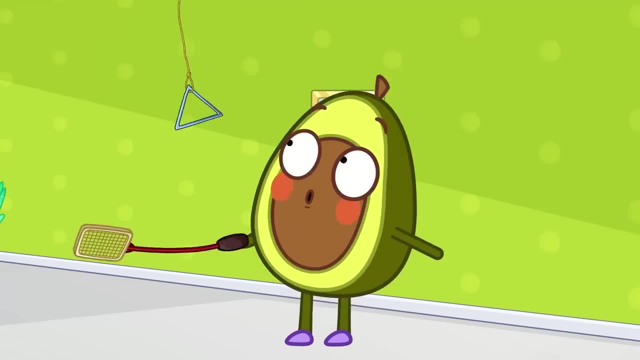 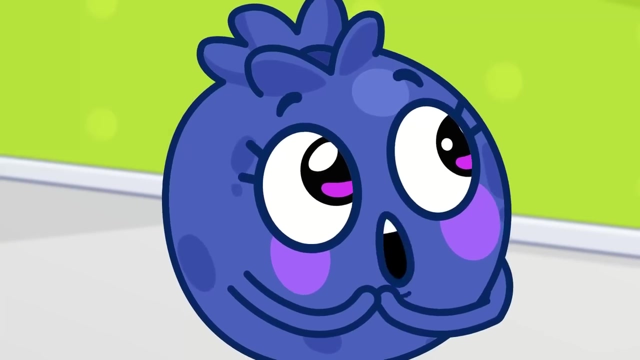 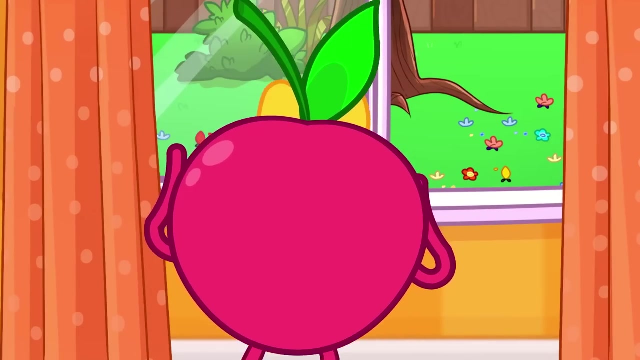 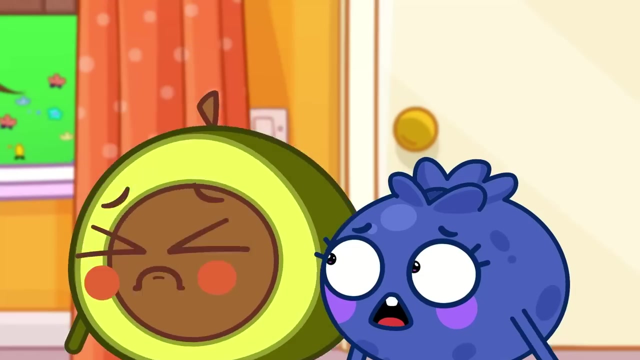 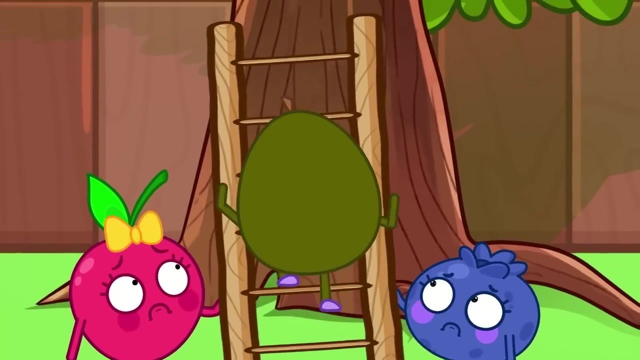 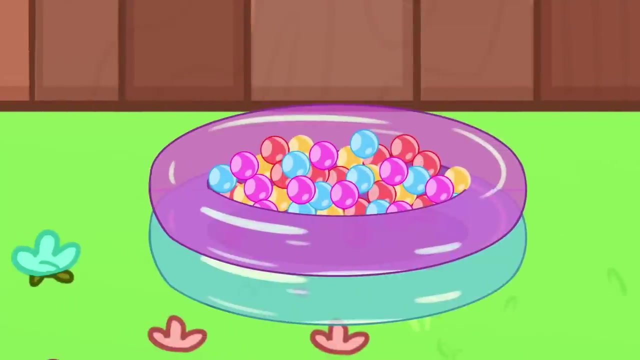 There, Pit, Now you can get it. Pit found Blueberry. Thank you There. Now the fly is gone. Penny's going to fall. Help me. You better hurry kids. The ball pit would be a safe place for Penny to land. 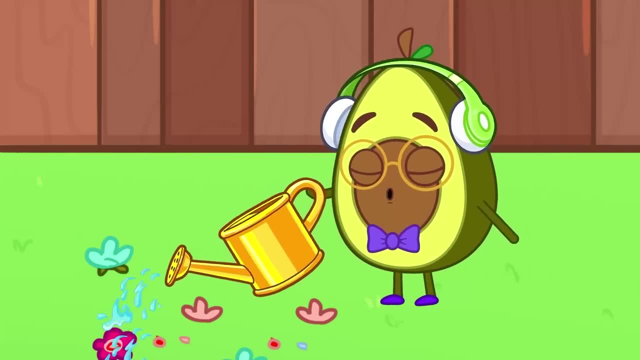 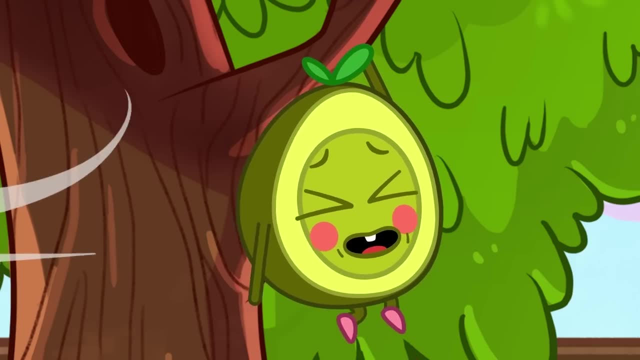 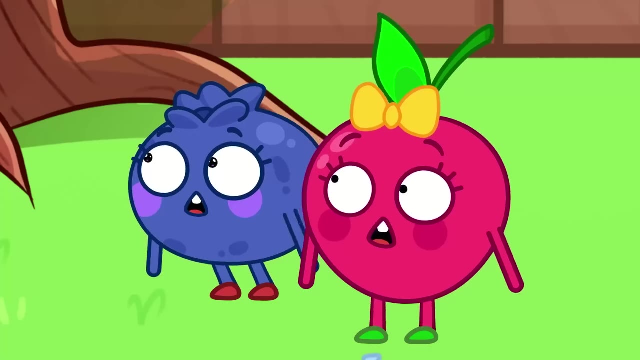 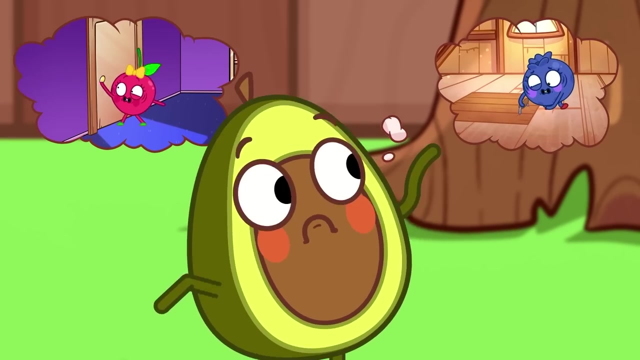 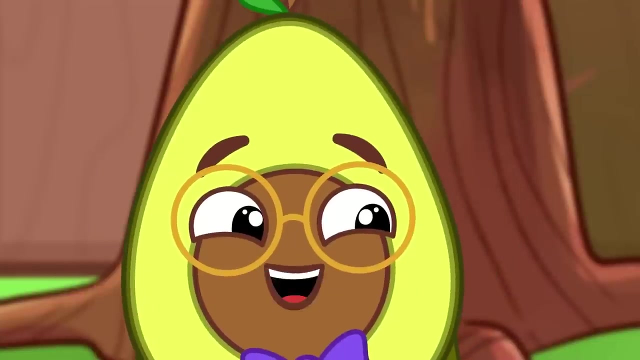 The wind blew it away. Daddy, the kids need you. Daddy arrived just in time. Don't hide in a tree- It's very dangerous. And don't hide in the attic or pantry. It's more fun to play safe. Let's play hide-and-seek together. 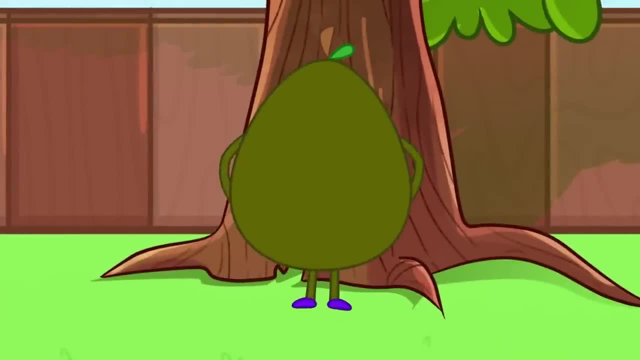 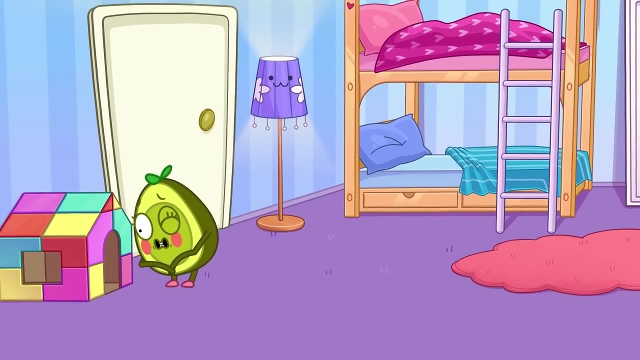 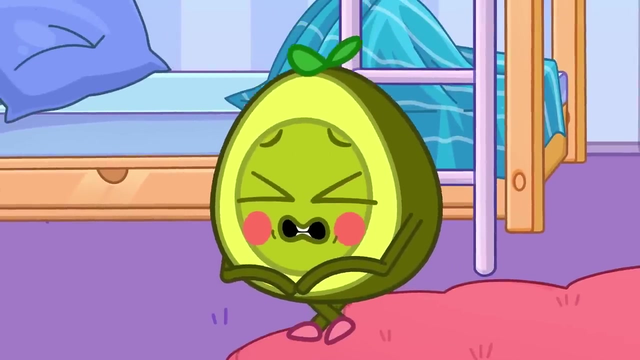 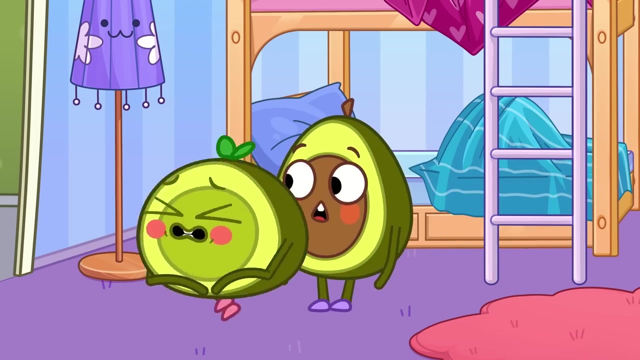 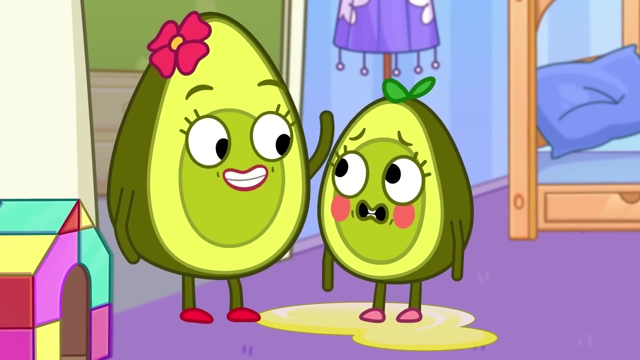 I will seek Ten, Nine. Have fun, everyone Eight. What is Penny looking for? Oh, she needs to pee but can't find her potty. Oopsie, Penny had an accident. Mom, You were too old to use the potty. 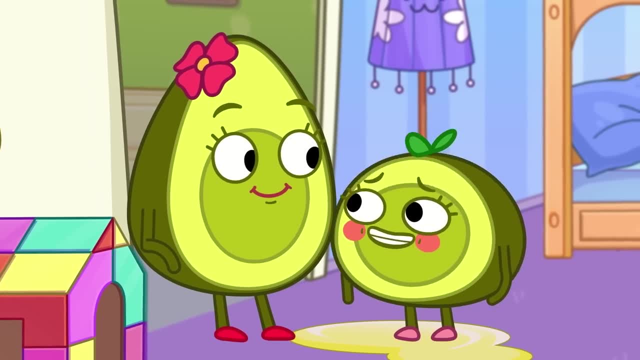 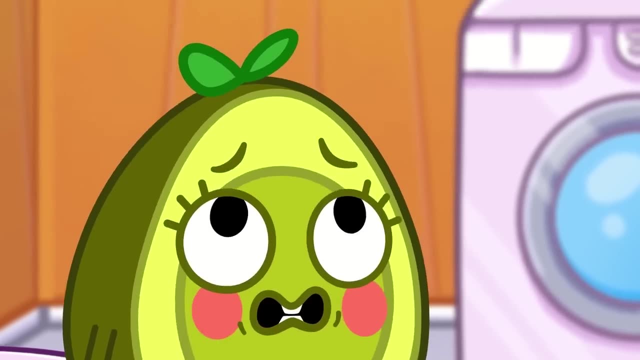 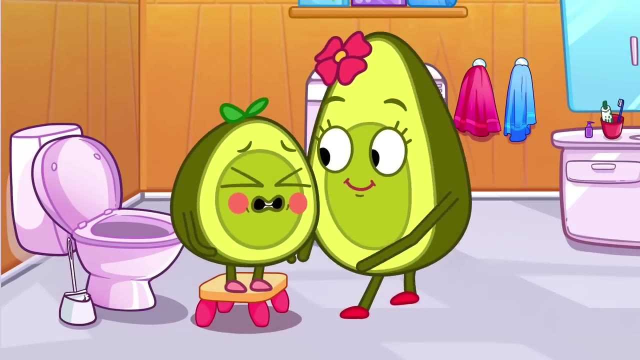 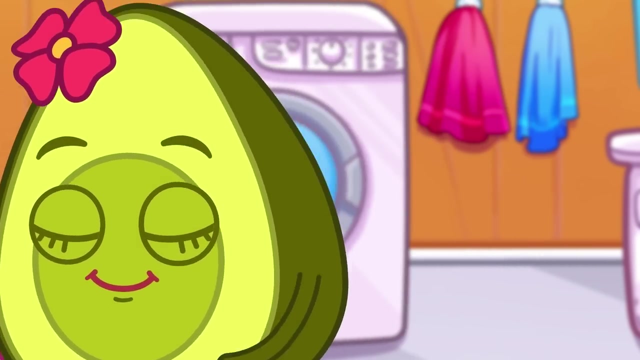 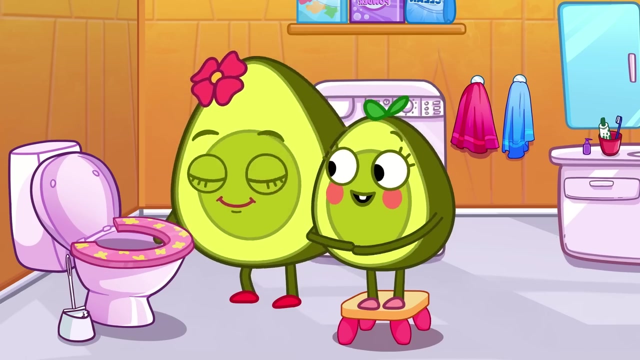 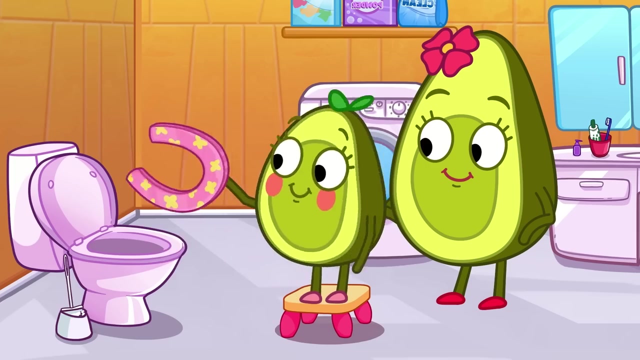 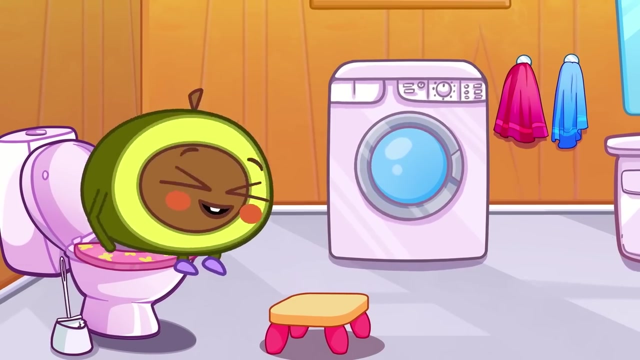 But Penny thinks big toilets are scary. She might fall in. Não, It's a special seat cover. You see, It's very simple. Now try it yourself And it really works. Pit flush the toilet, please, Ah. 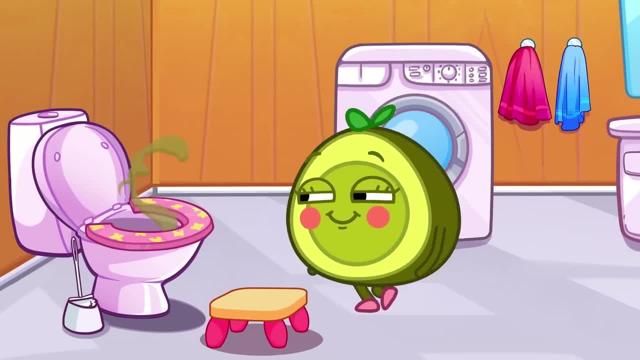 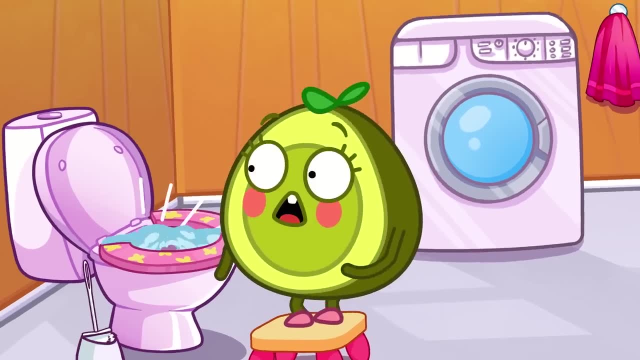 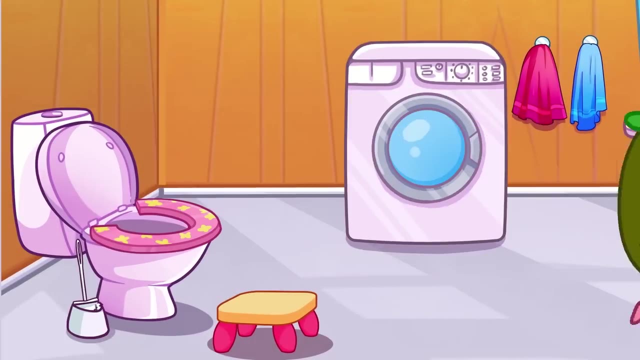 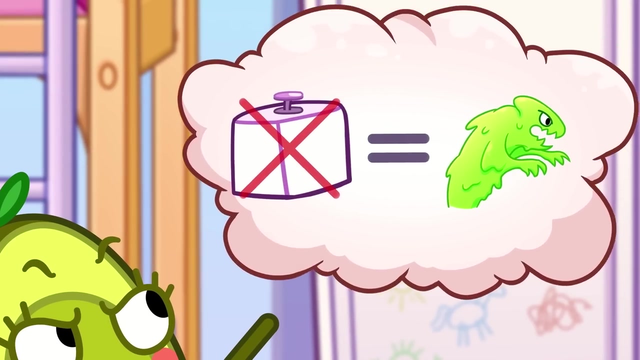 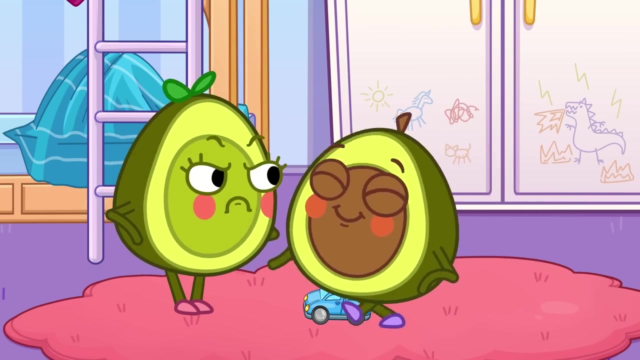 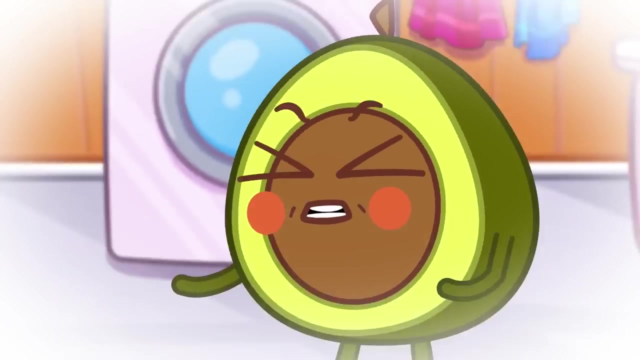 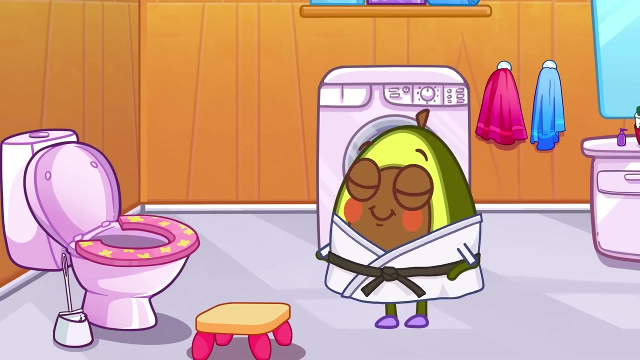 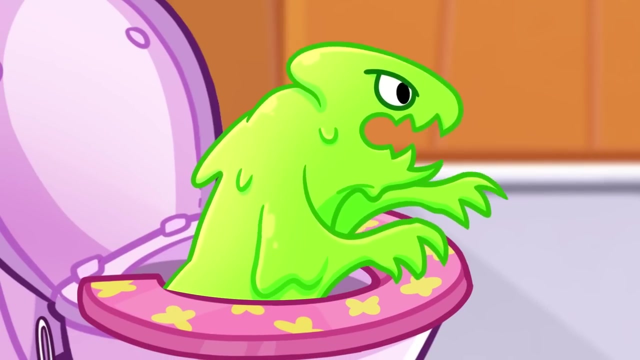 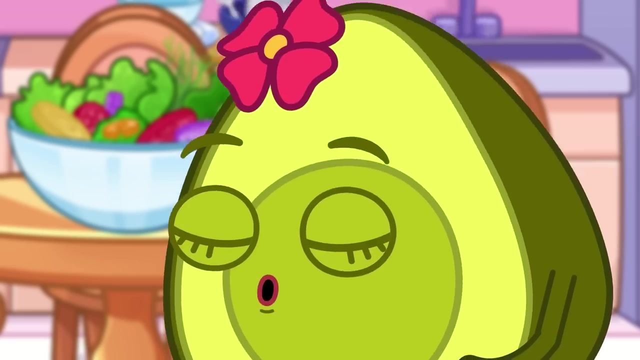 He left a stinky mess inside. Now Penny thinks there's a toilet monster. Pit, by not flushing… You awakened a toilet monster Monster. you say Pit's not afraid at all, But Penny is. Oh, Ah, What's happened? 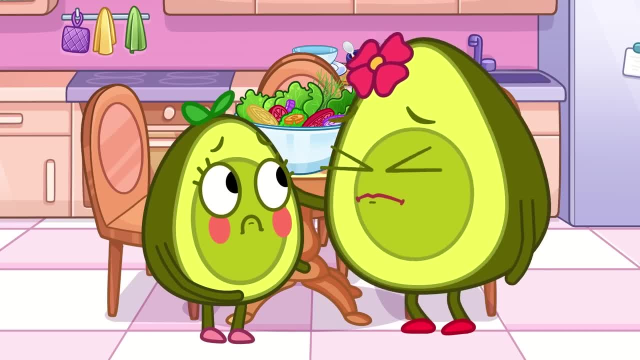 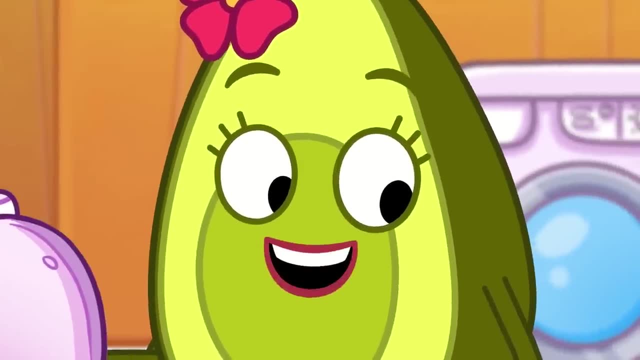 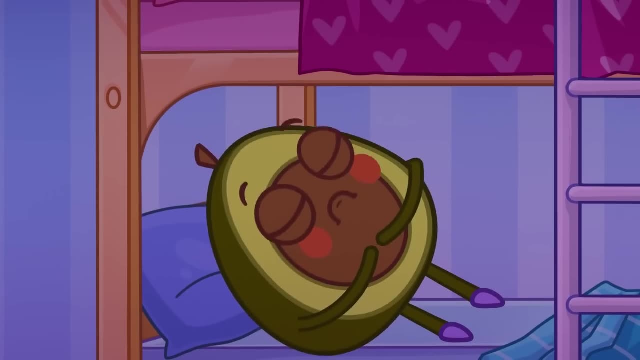 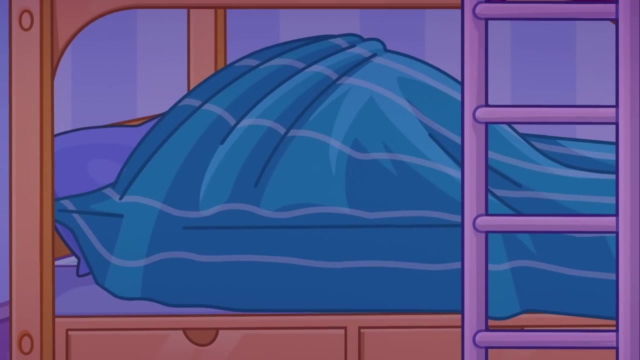 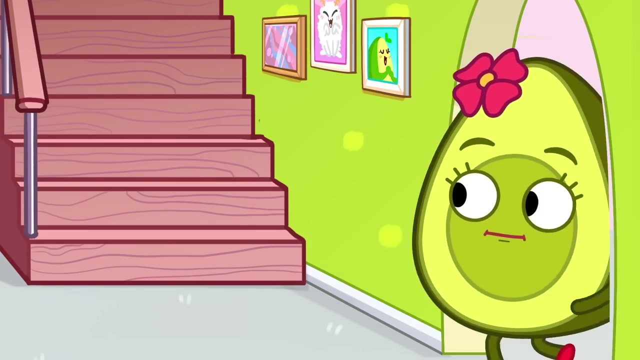 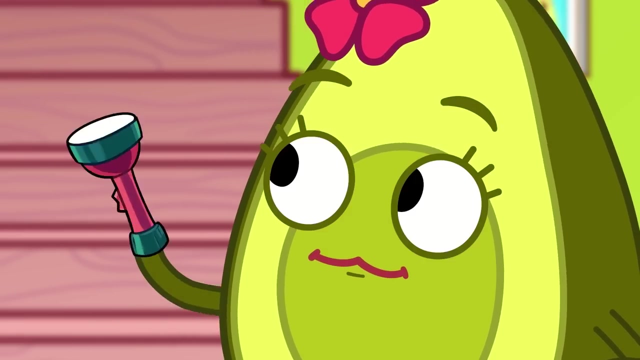 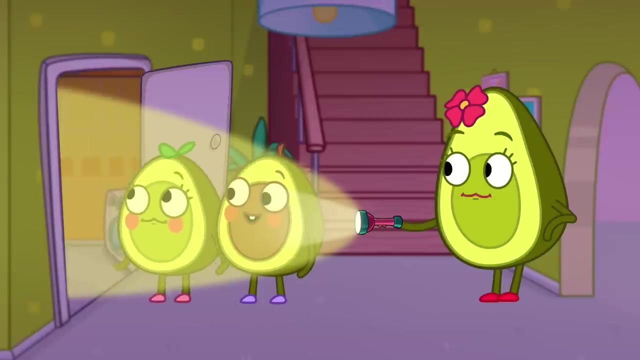 I'm afraid of the toilet monster. It's not a monster, It's just the sound of the toilet flushing. Now Pit needs the toilet, But he's scared… Oh, there are no monsters There. Now everyone is ready for bed. 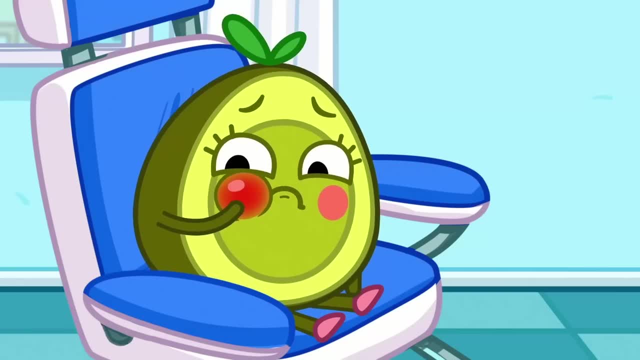 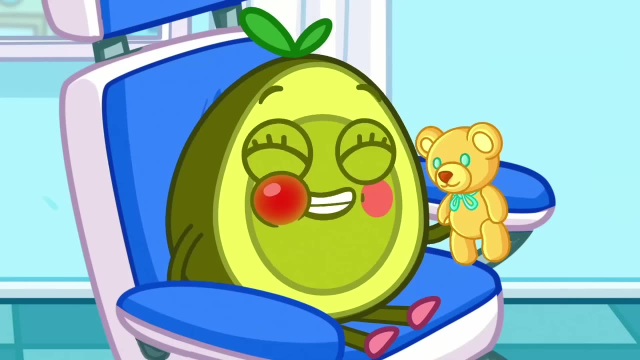 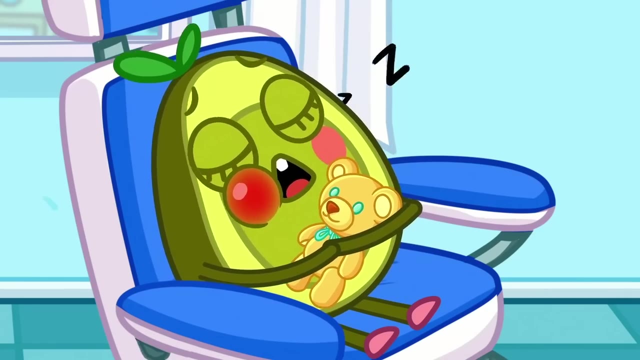 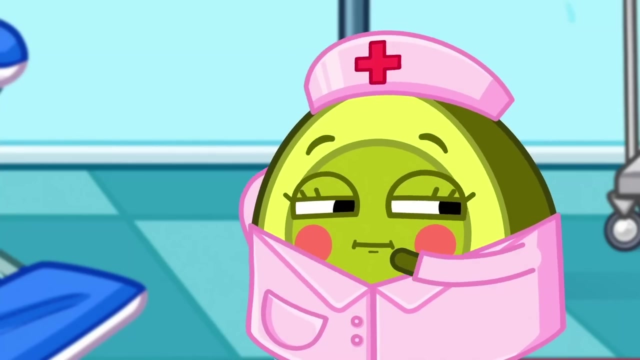 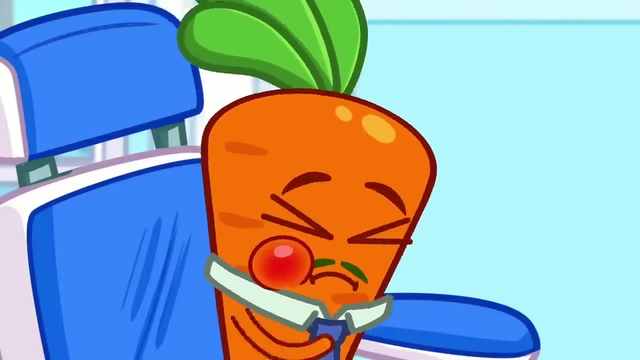 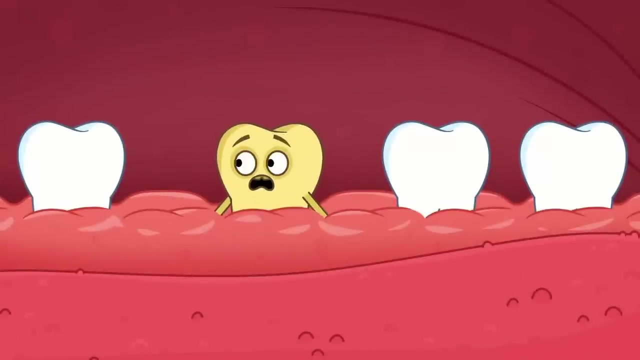 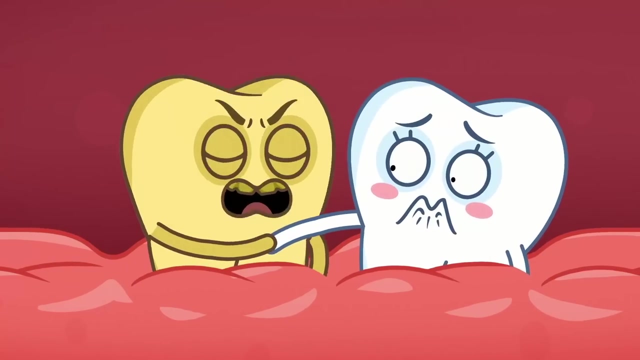 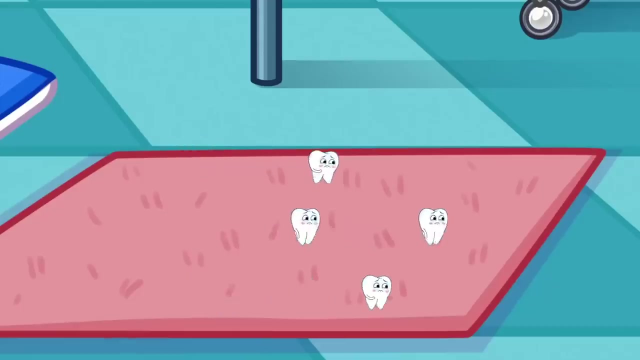 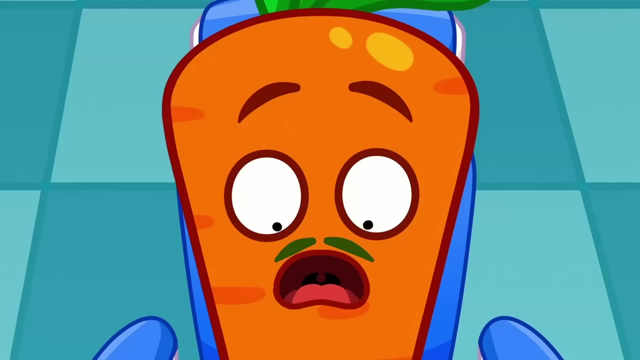 Nighty-night Penny needs to see the dentist. Maybe a teddy bear will help her relax. Now she's dreaming she's a dentist. Open your mouth. There's a cavity inside The teeth. don't want to turn bad. No. 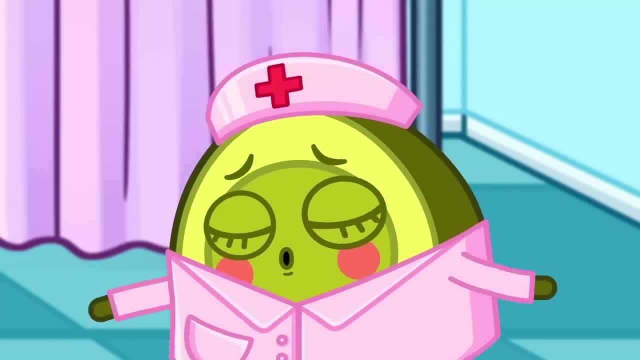 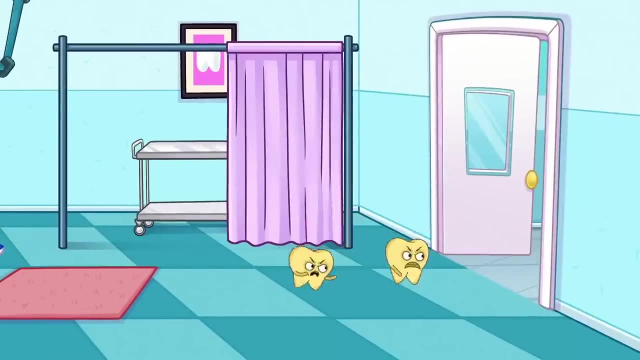 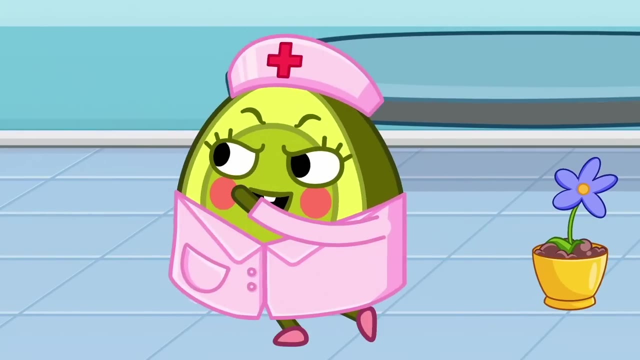 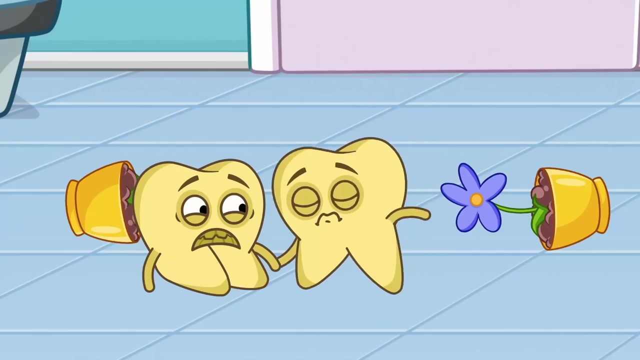 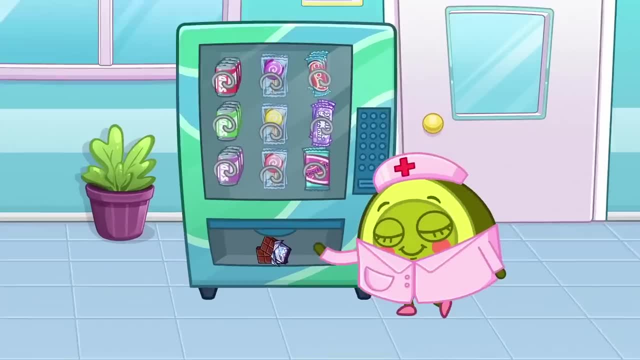 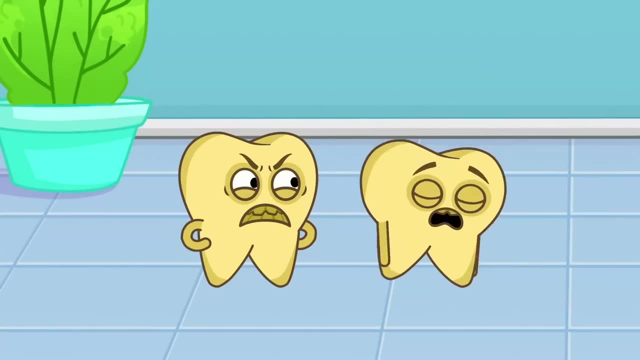 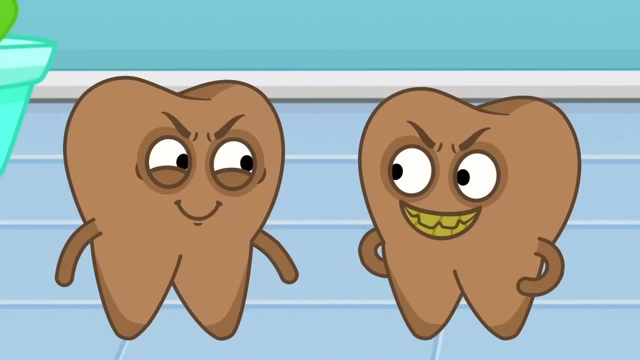 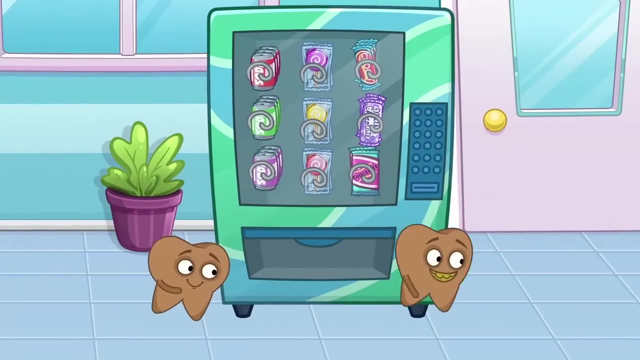 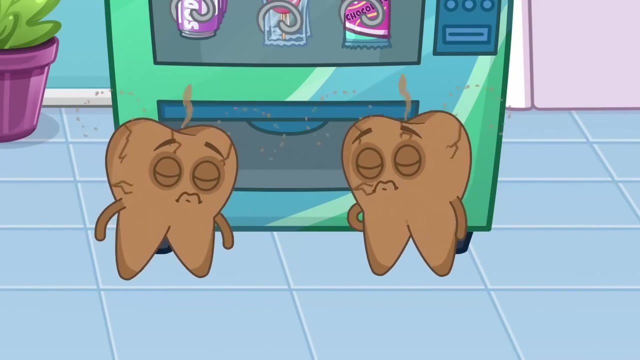 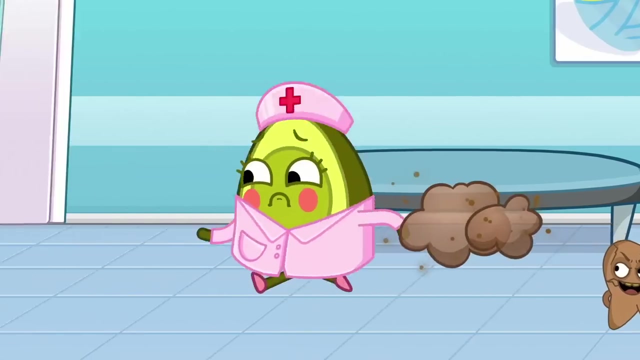 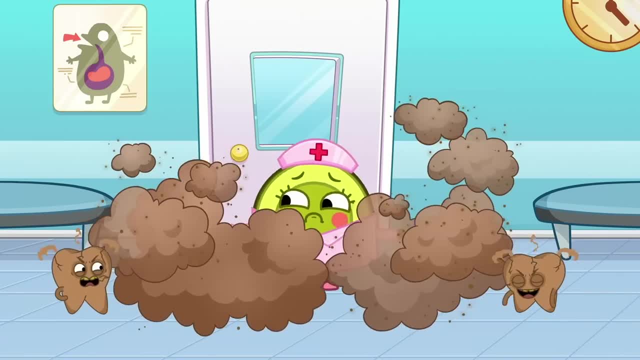 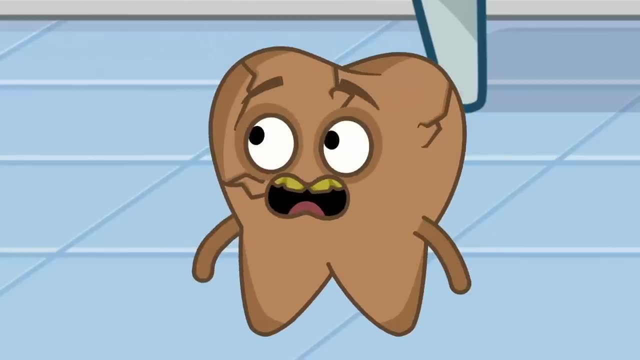 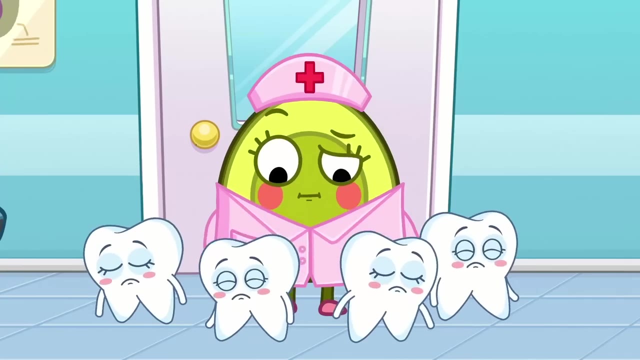 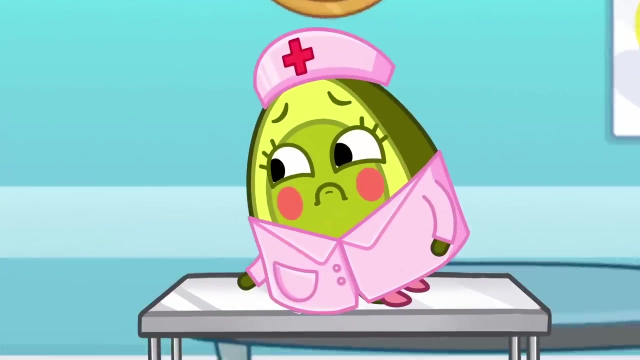 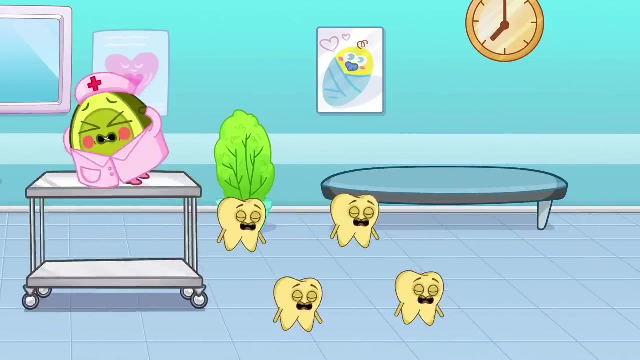 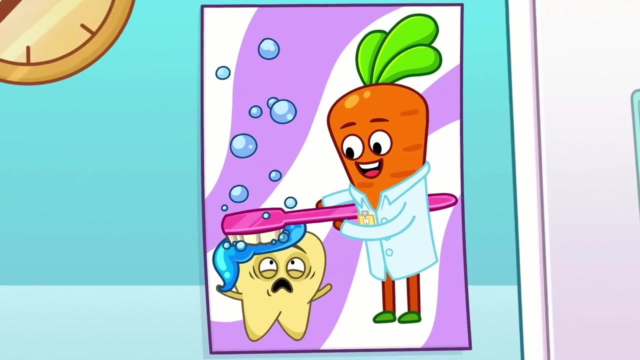 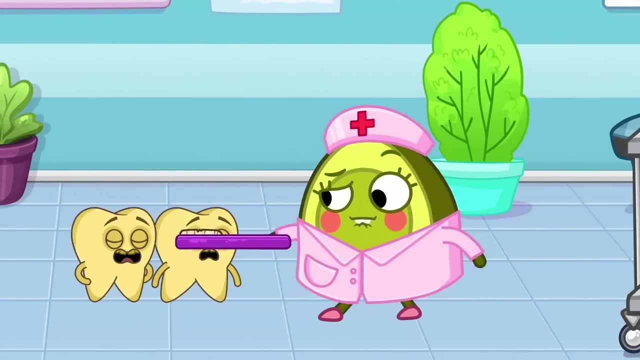 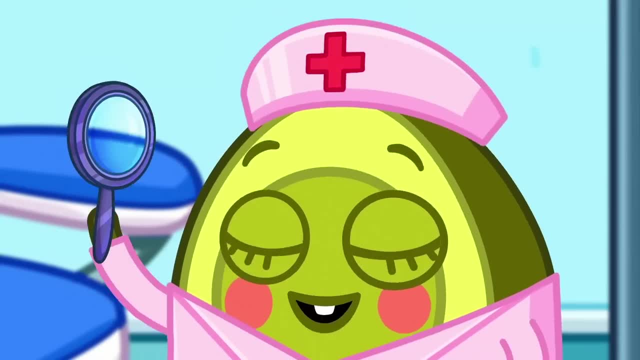 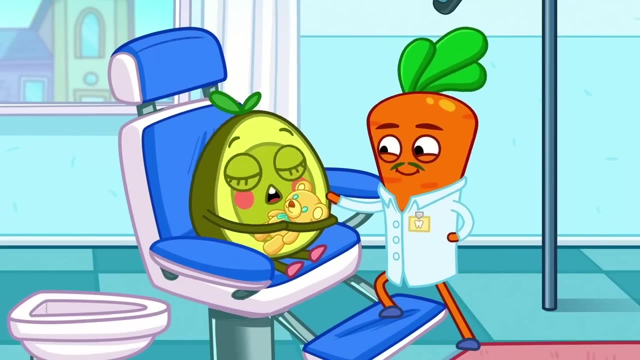 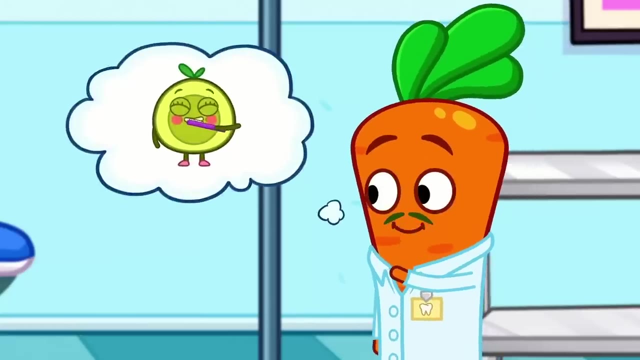 There, Mr Carrot has his teeth back. Wake up, Penny. All done, Your teeth are healthy. Good job, Penny. And to keep your teeth healthy, brush them with a toothbrush. Eating too many sweets is bad for your teeth. 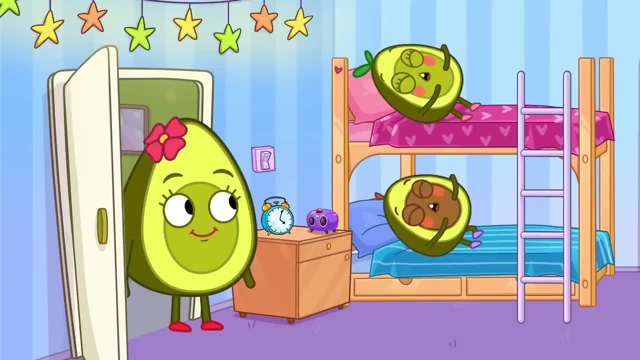 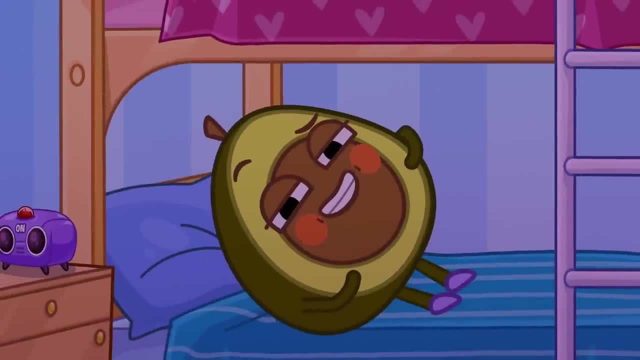 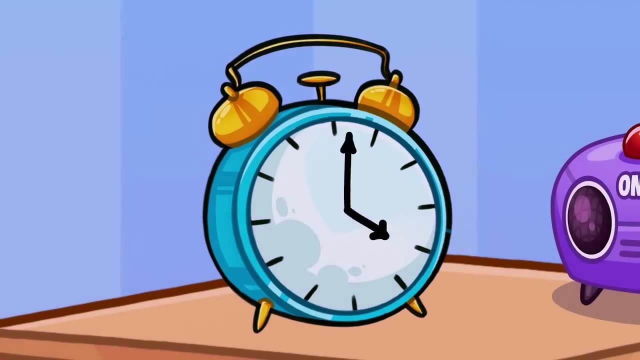 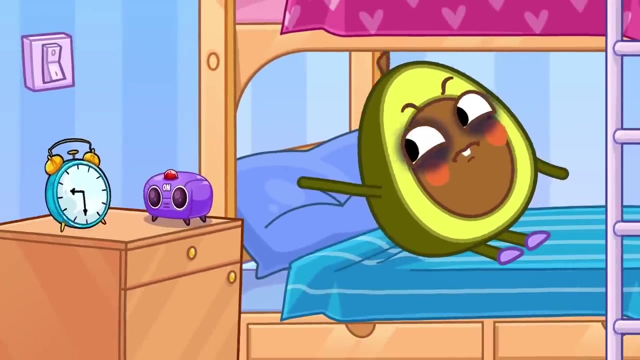 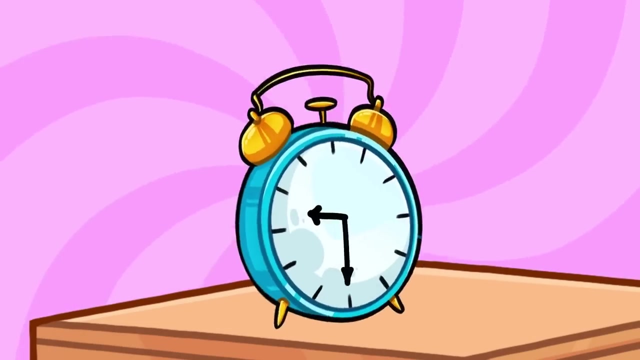 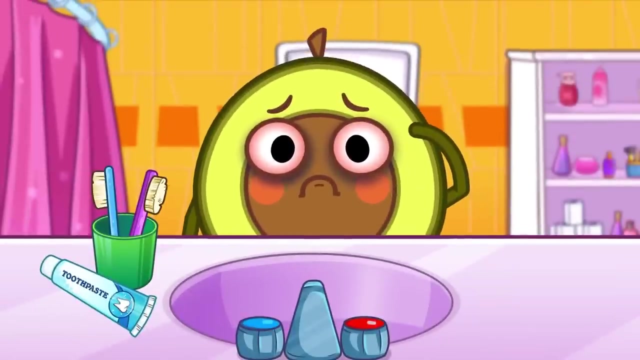 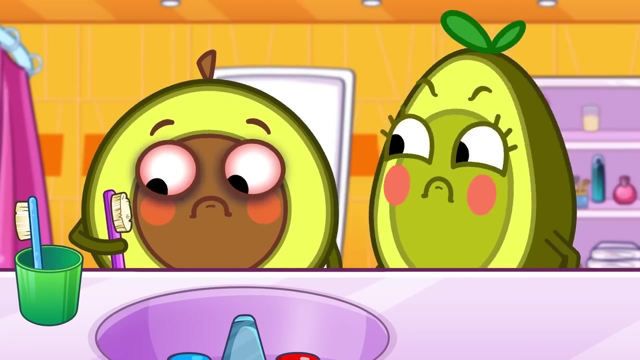 Thank you, Dr Carrot. It's bedtime for Pit and Penny, But Pit is only pretending He just wants to play video games. Oh no, Pit has been up all night And he's having trouble seeing clearly. Woo, Wait, That's Penny's toothbrush. 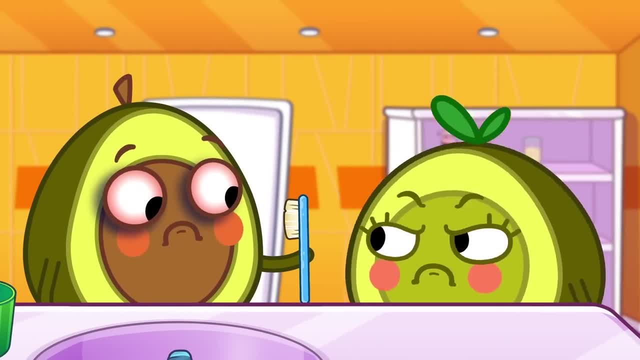 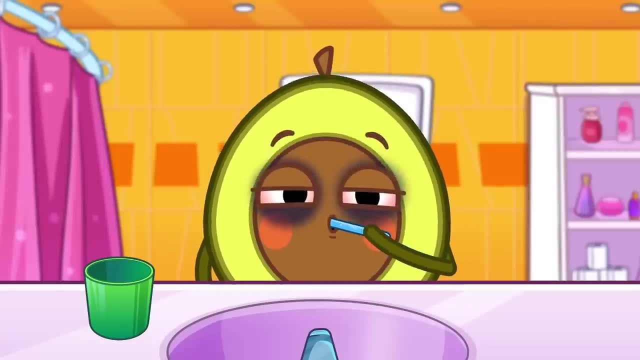 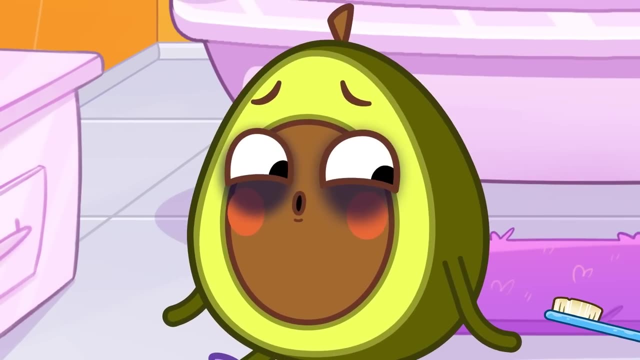 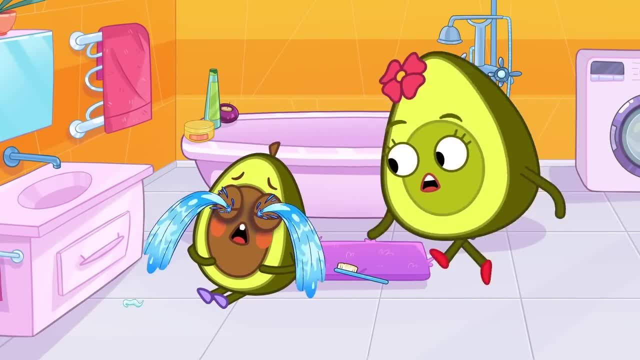 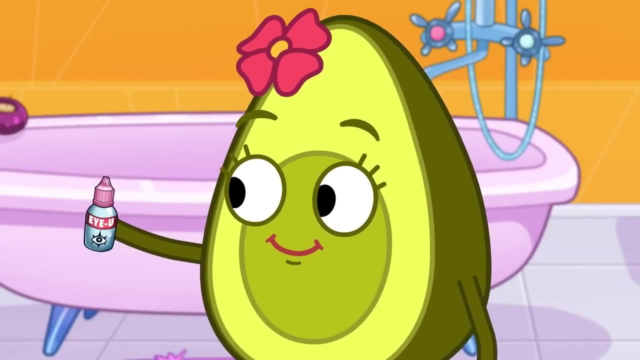 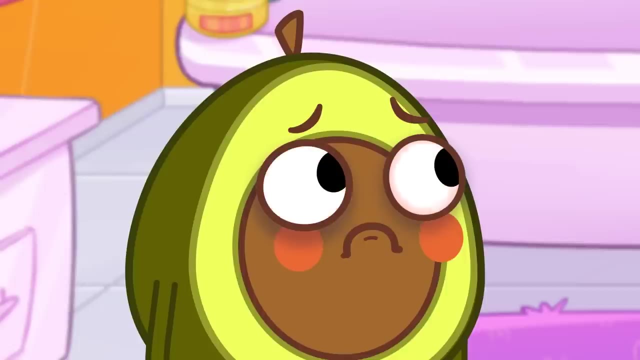 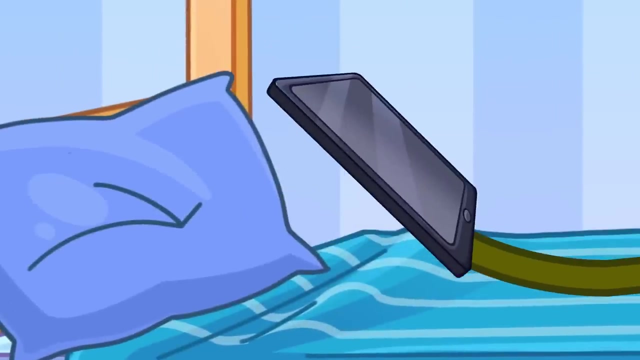 Hmm, Hmm, Hmm, Hmm, Tell, Tell Mommy what's wrong. Pit, My eyes can't see. Mommy knows what to do. I can see everything. Pit was playing games last night. Hehehehe, Hehehehe. 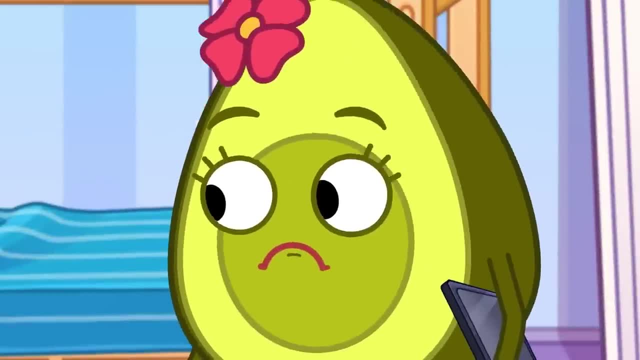 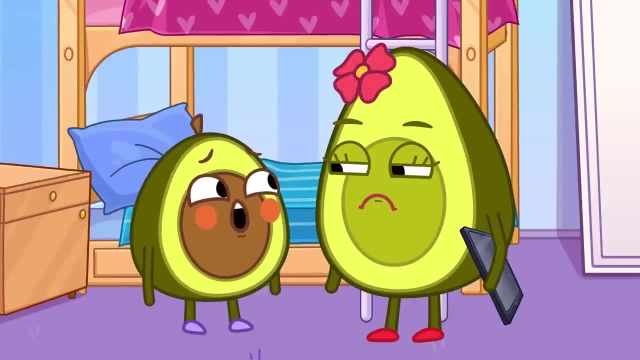 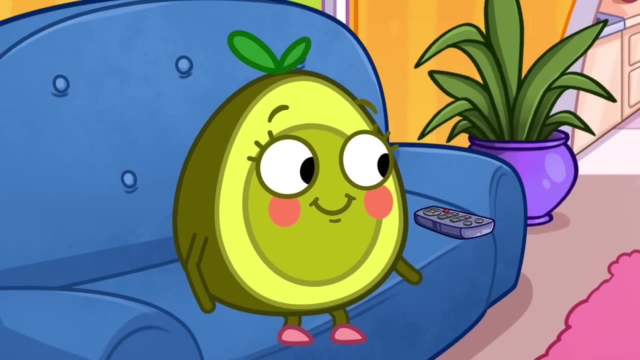 Oh Yay, Hmm. Playing video games at night damage your eyesight. Eh, I won't do it again. Oh, Hehehe, Hehehe. Penny wants to watch TV. Hehehe, Hehehe, Hehehe. 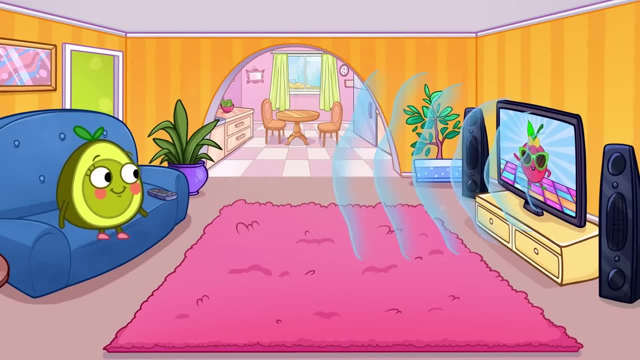 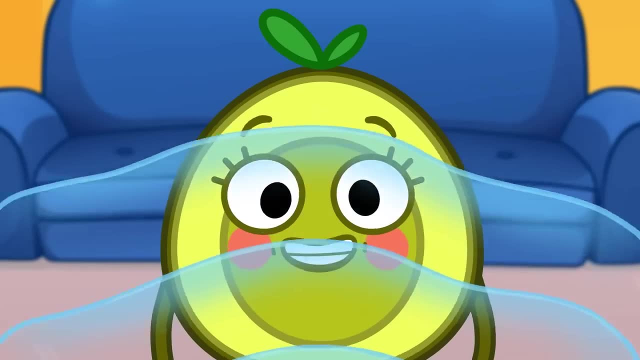 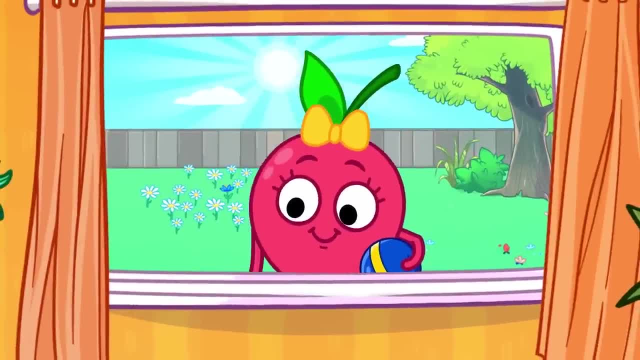 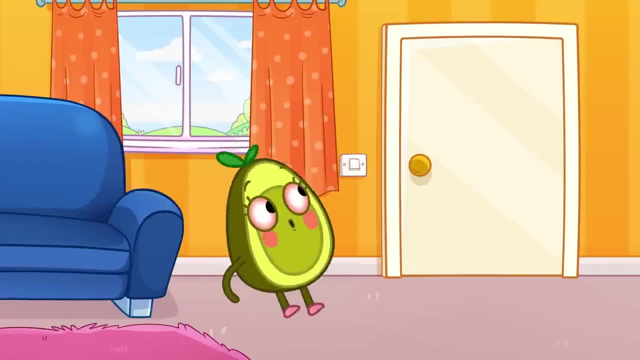 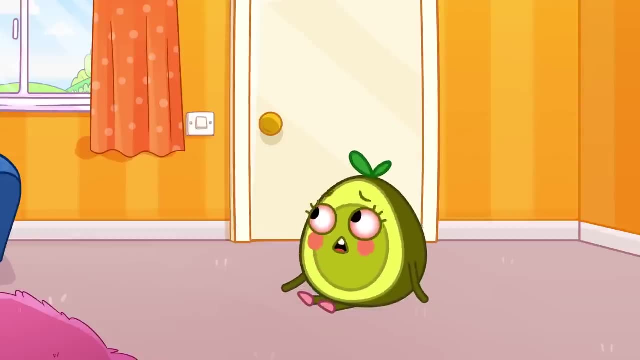 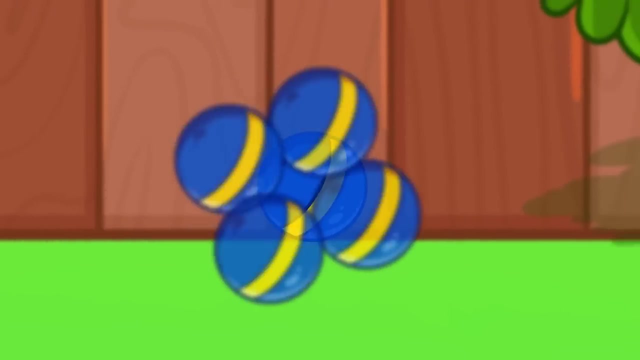 Huh… Look, Cherries come to play. Oh, Oooh, Ohh. But now Penny's eyes are blurry. Ah, Oh, Oh, Penny loves playing catch. Haha, Whew, These eyes are amazing, All right. 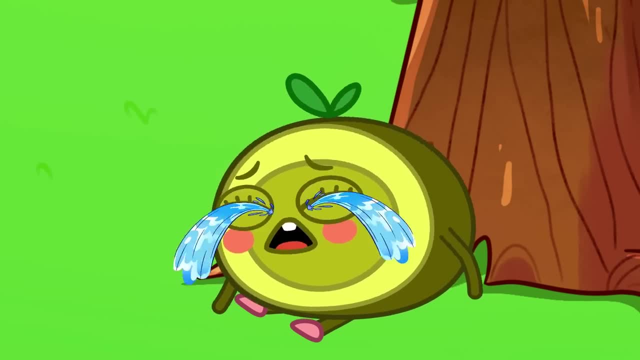 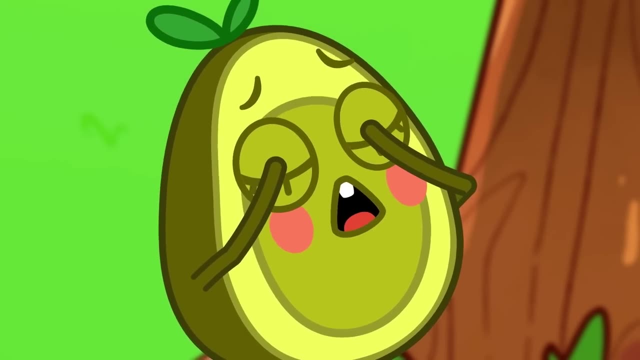 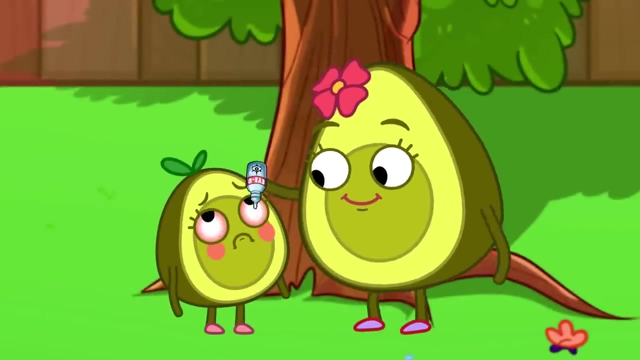 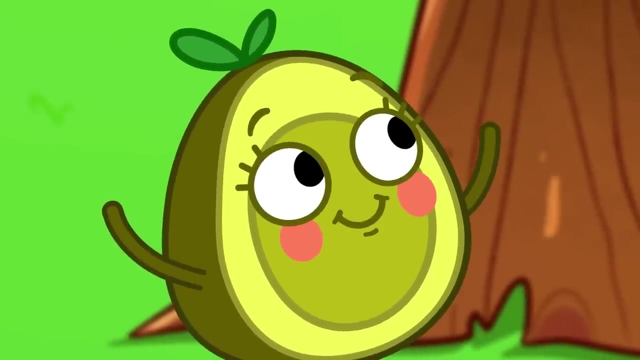 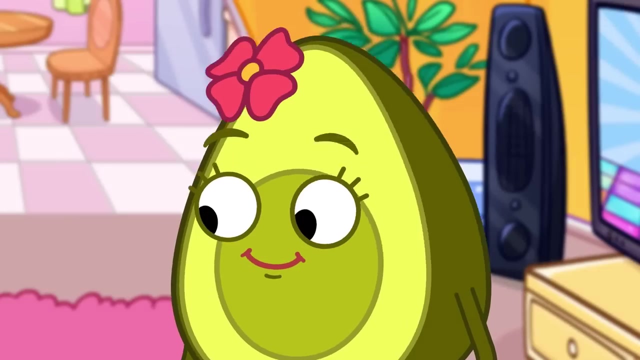 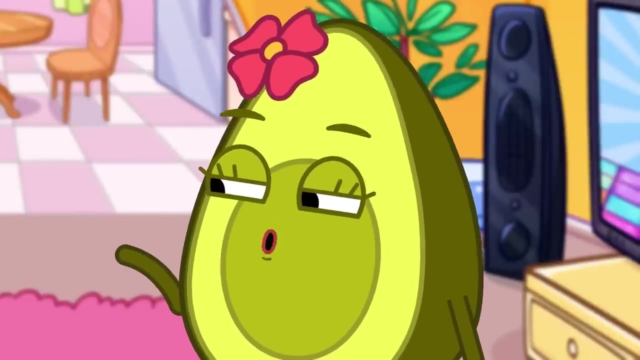 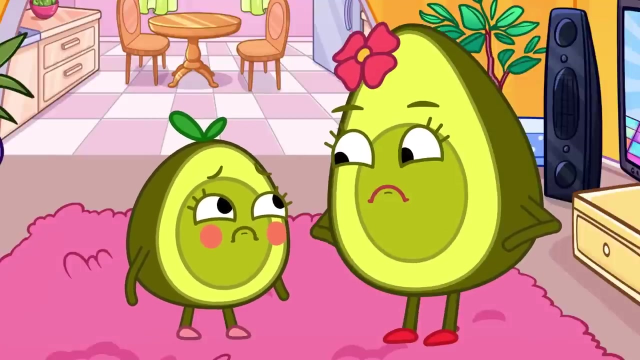 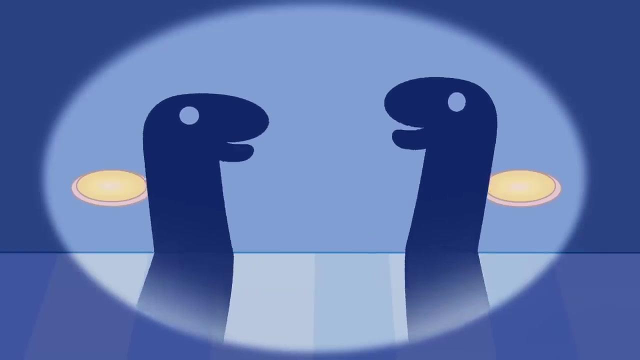 Go. My eyes can't see, Don't worry, Mommy has some eye medicine. I can see everything. Mommy knows what Penny did wrong. Watching TV from too close ruins your eyesight. I won't do it again. The kids want a flashlight fight. 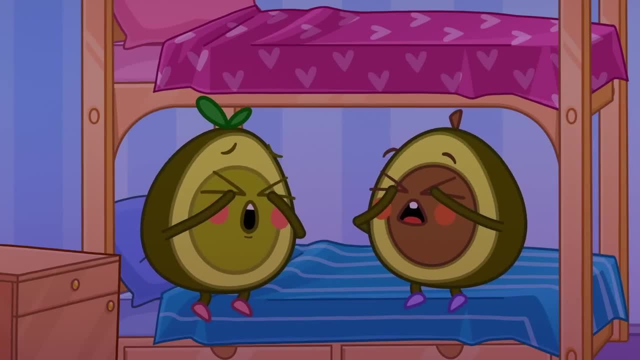 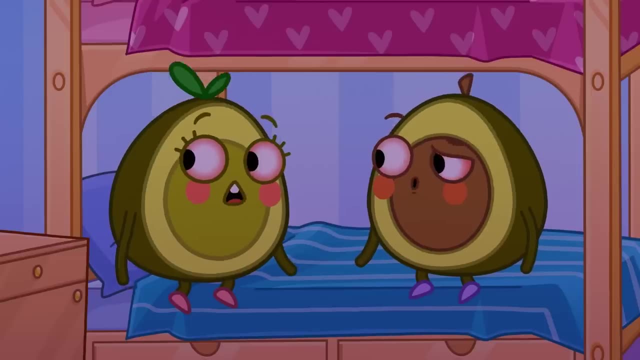 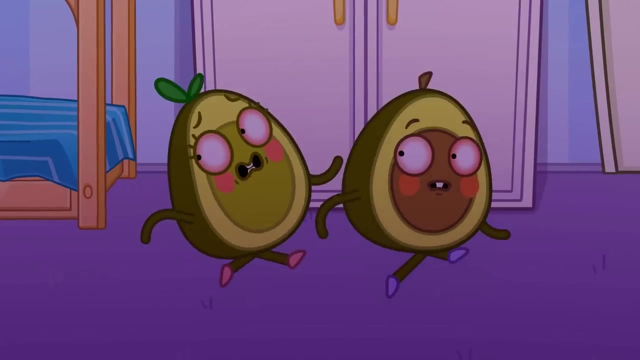 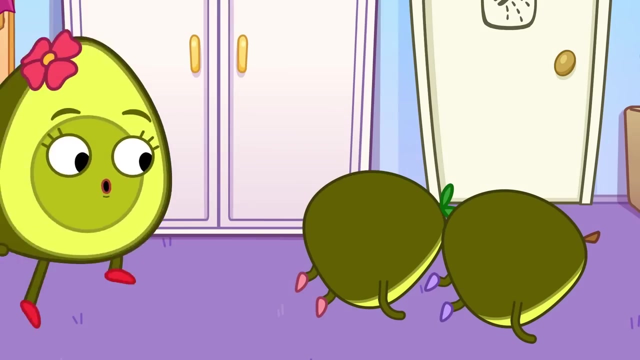 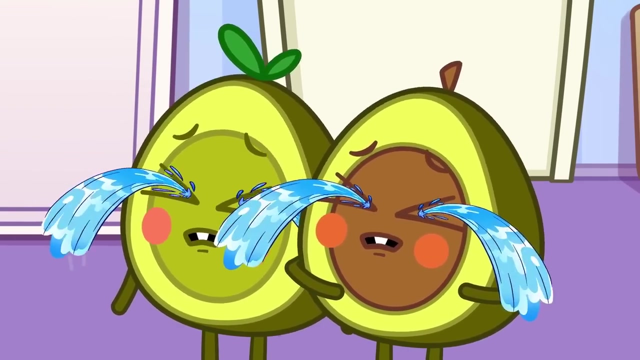 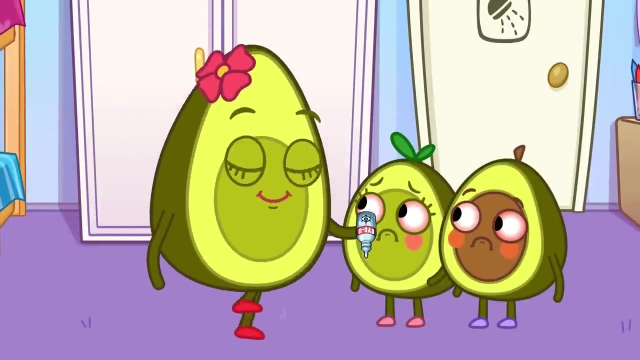 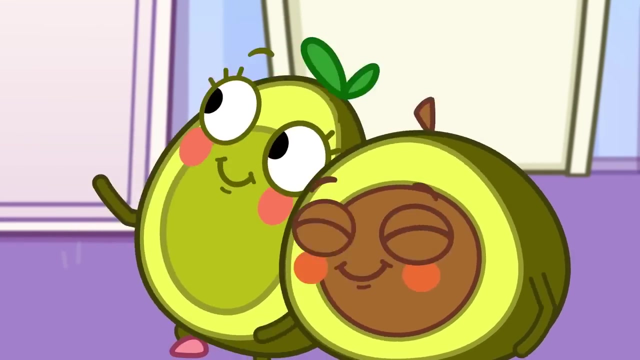 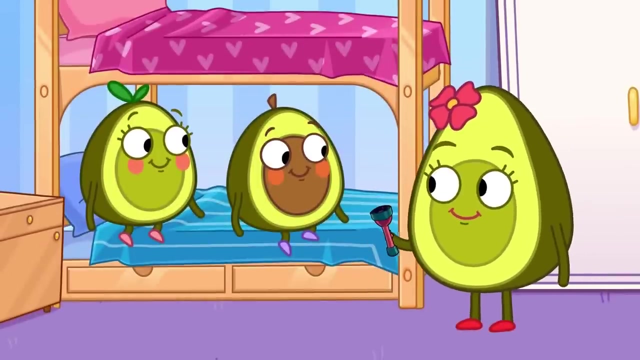 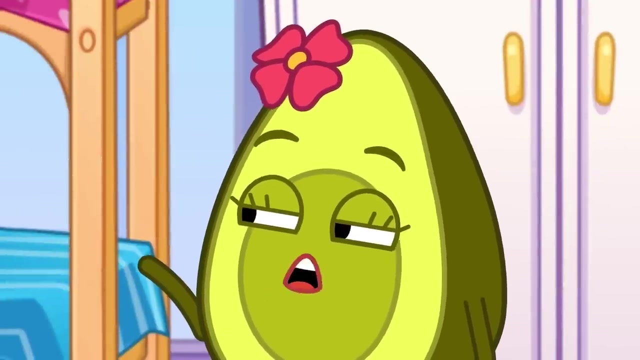 They think Mommy's a monster Kids. it's just Mommy, We can see everything. Here are some more eye drops. That's much better, Thank you. Our eyes are very sensitive, So don't shine light directly into them. 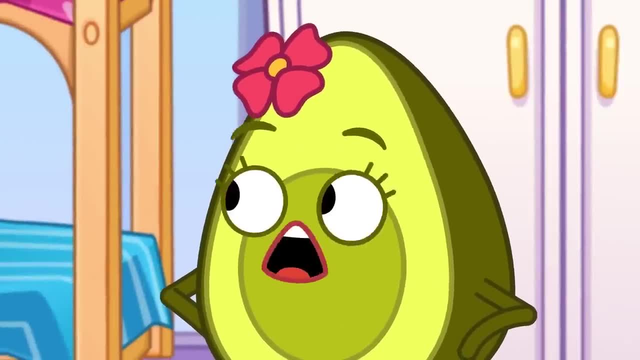 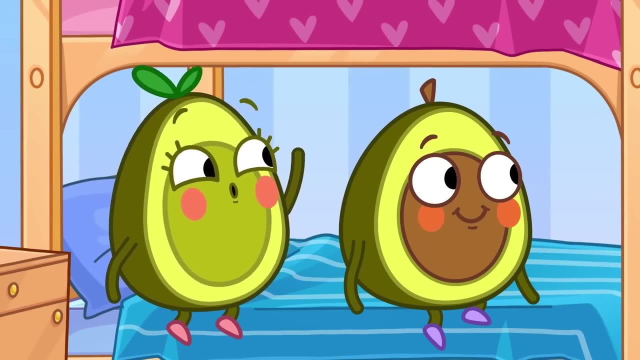 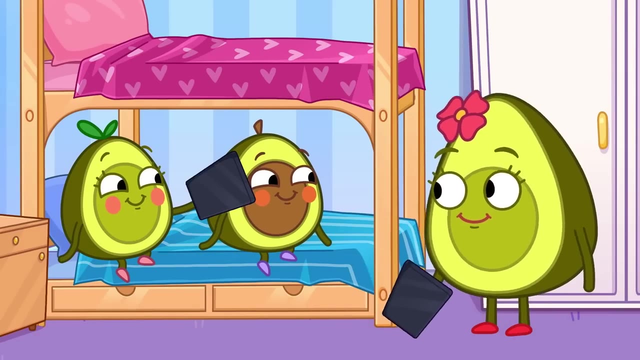 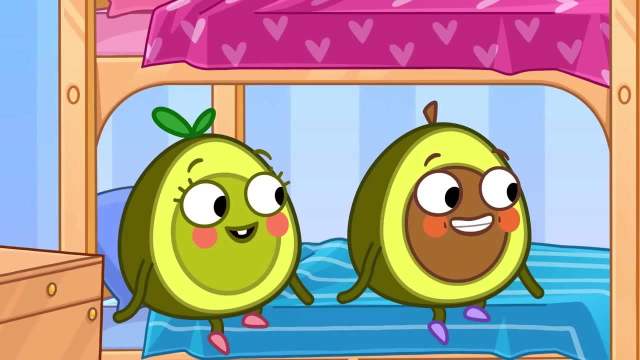 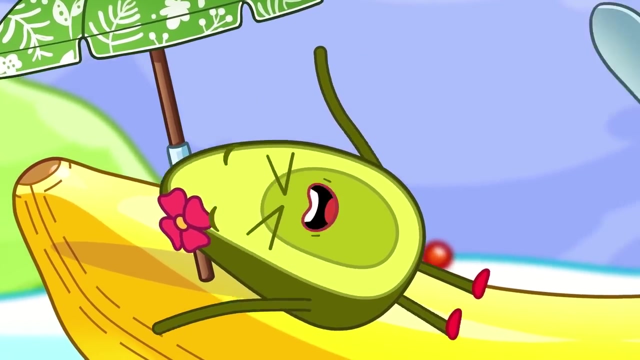 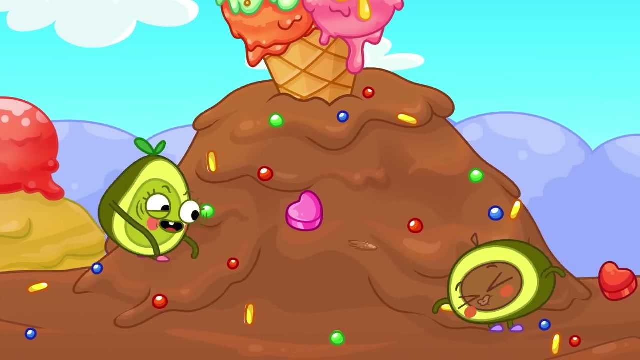 And don't sit too close to TVs and other screens. I will always keep my eyes healthy, Me too. Me too. Now, your eyes will stay healthy. Yay. Mommy and Daddy are relaxing on a banana boat, While Penny and Pip play on a hill of chocolate. 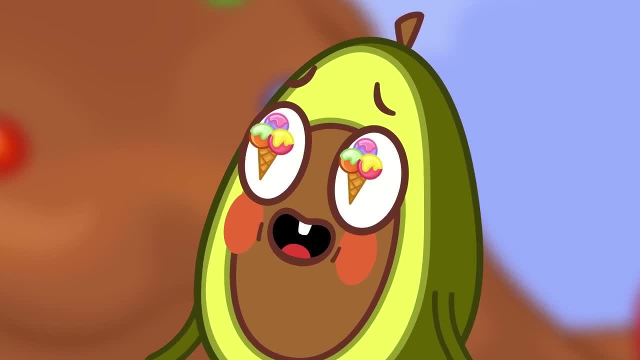 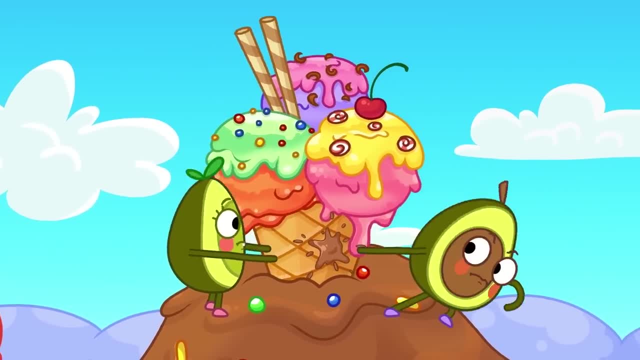 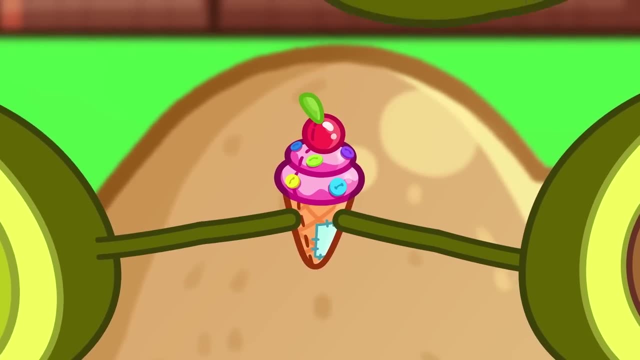 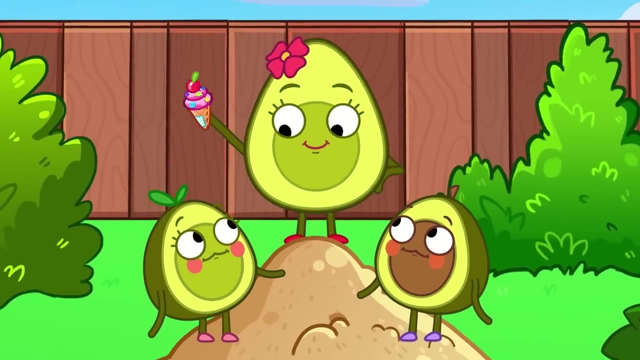 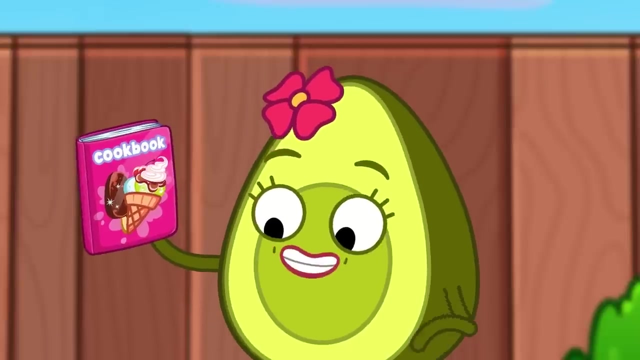 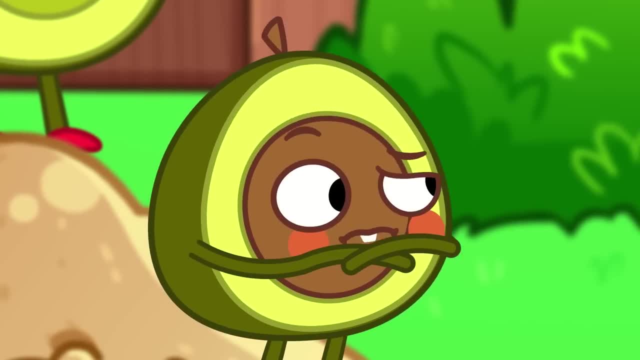 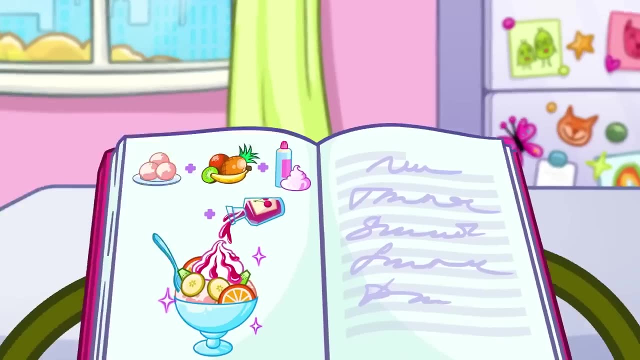 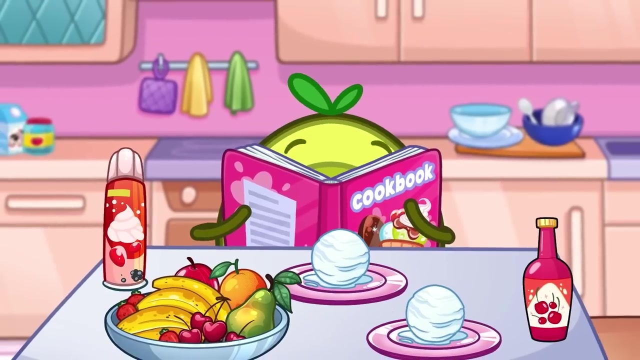 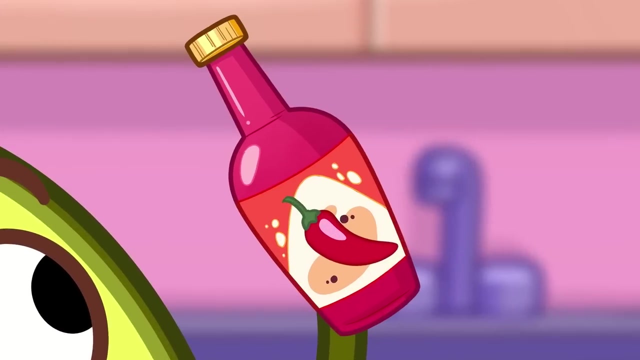 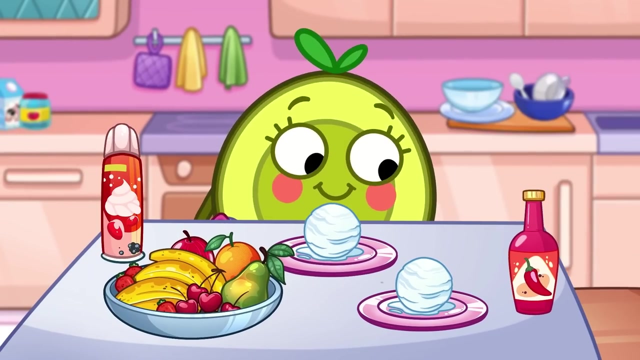 Penny loves the idea. What about you? Pit Cooking is farming. What will Penny make? A sundae? Oh no, He switched the cherry topping with hot pepper sauce. Oh no, He switched the cherry topping with hot pepper sauce. Careful Penny. 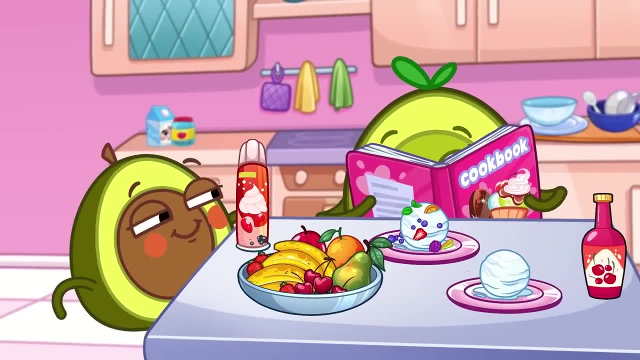 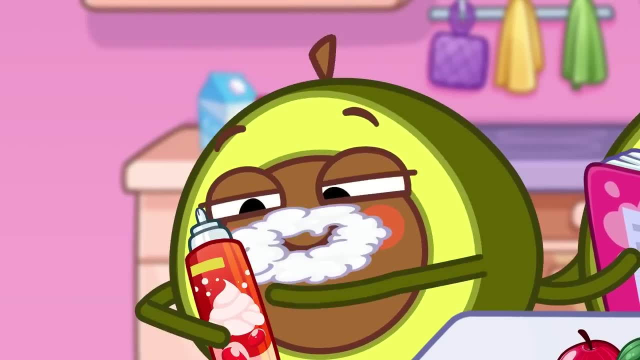 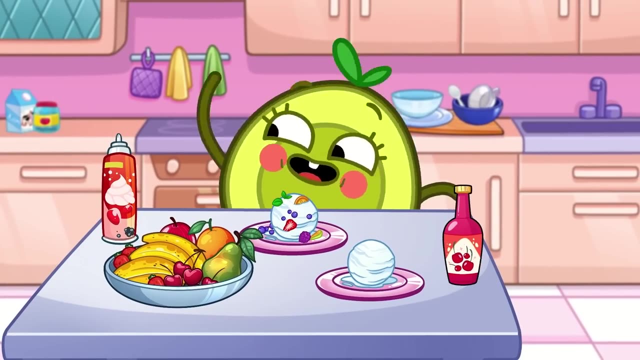 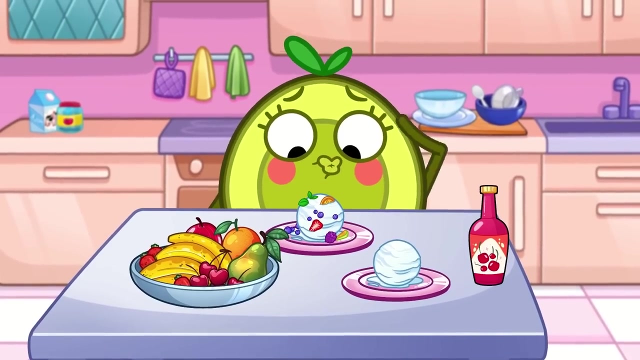 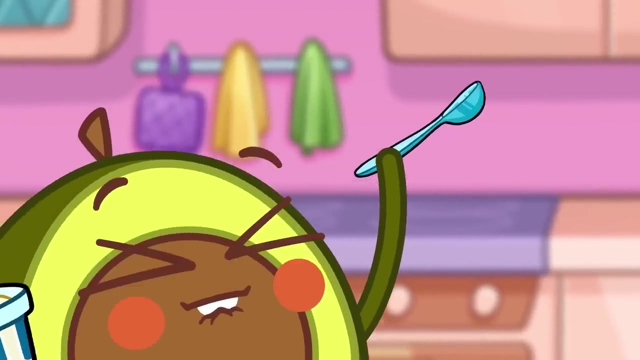 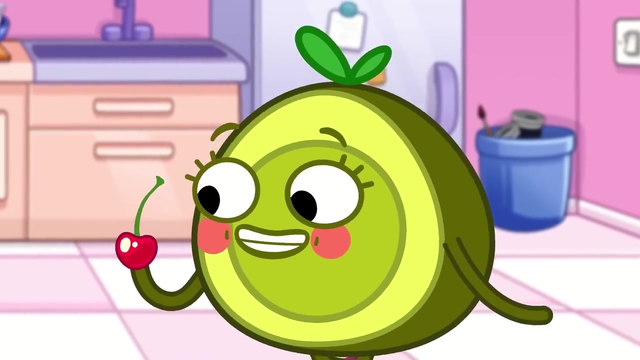 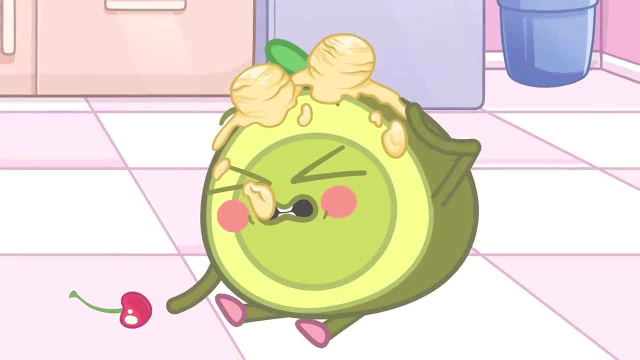 What else does Penny need? What else does Penny need? Pit? just ate all the whipped cream. There's none left for Penny. Now. what is Pit up to Now? what is Pit up to Now? what is Pit up to? Look what you did, Pit. 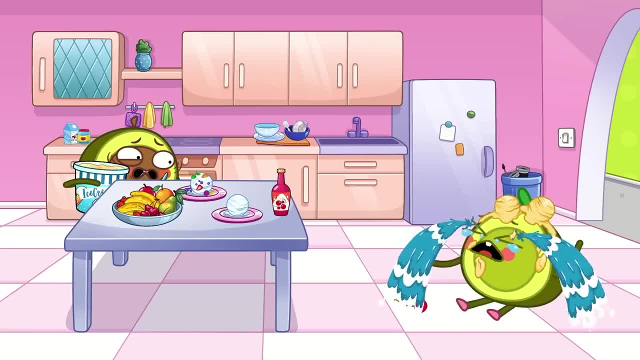 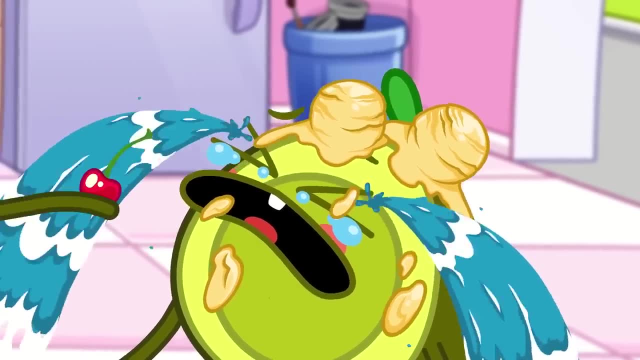 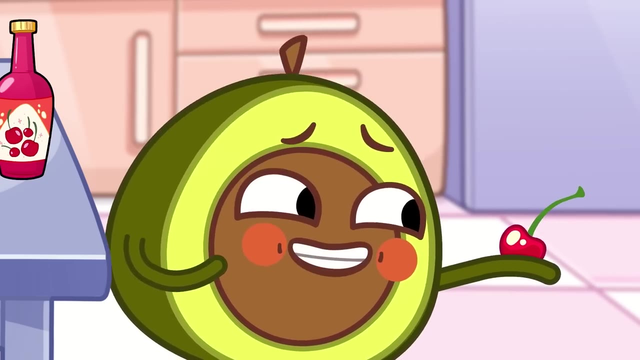 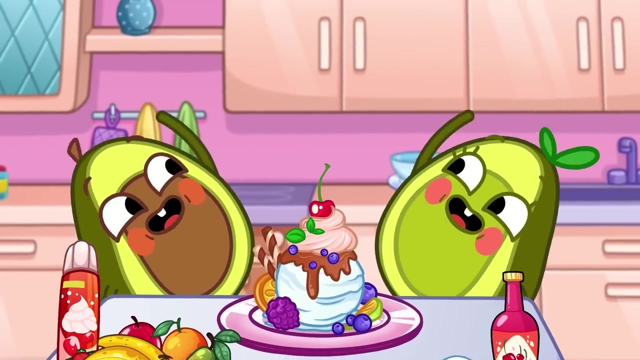 Look what you did, Pit. Pit has something to say. Pit has something to say, Penny, I'm sorry. Let's make ice cream together. Let's make ice cream together. Let's see what Mommy and Daddy think. Let's see what Mommy and Daddy think. 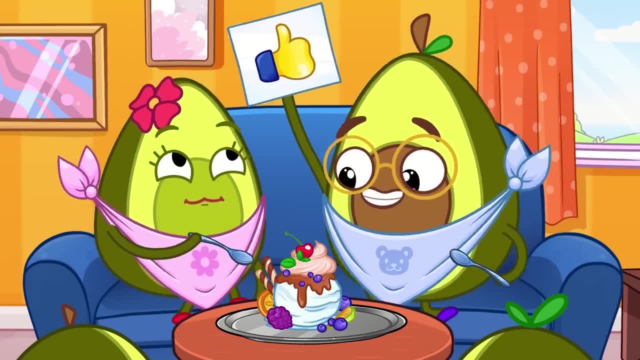 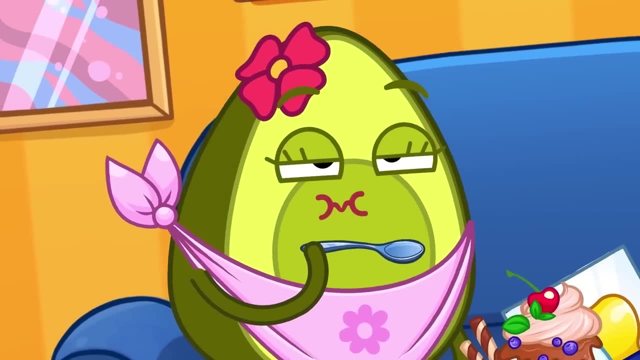 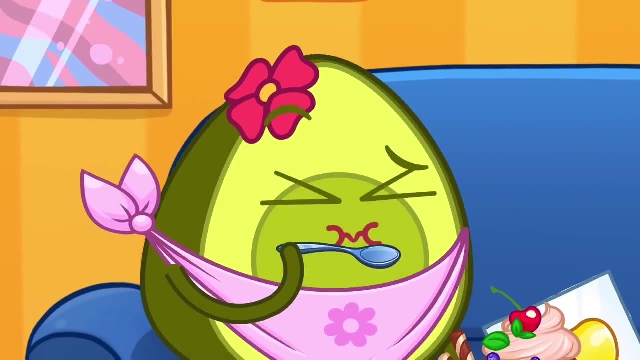 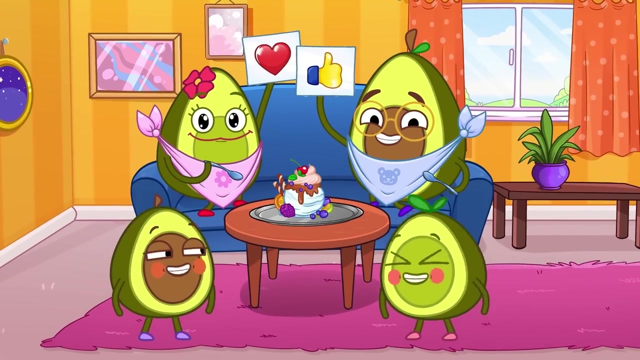 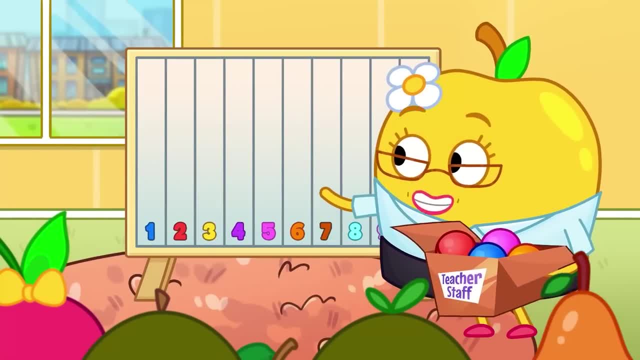 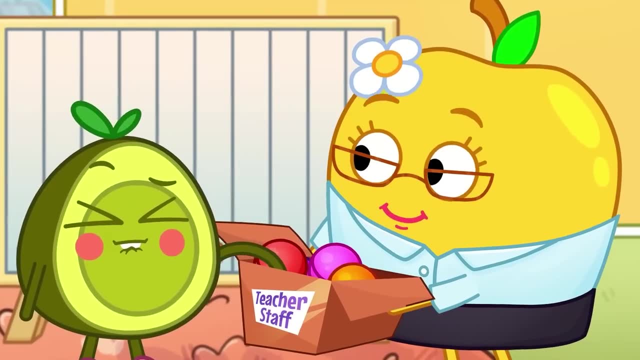 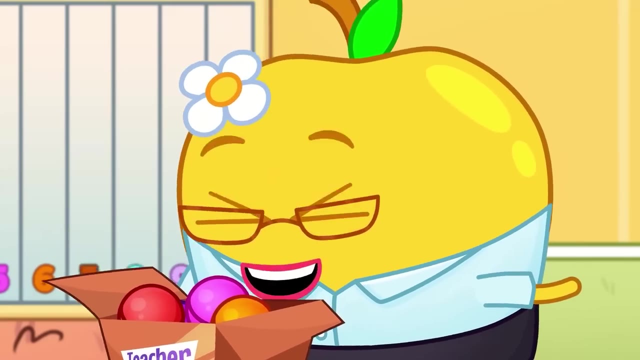 Hey kids, Let's learn numbers. It's okay Pit. It's okay Pit. Numbers are fun to learn. What number will Penny pick? Do you know the number? Oh, it's number one. Now put it on the board, Penny. 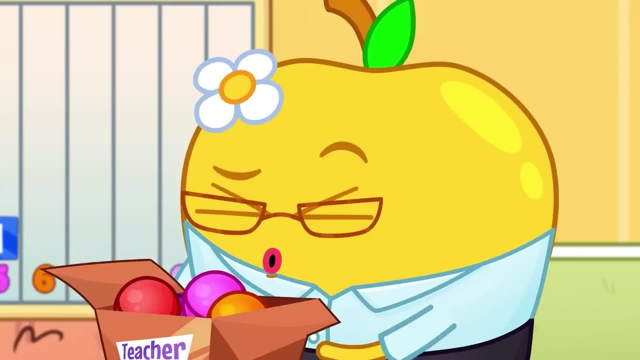 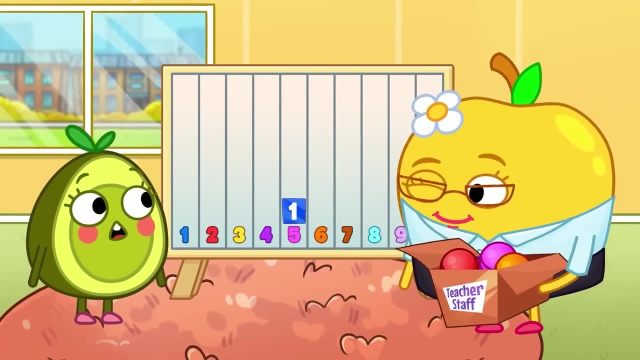 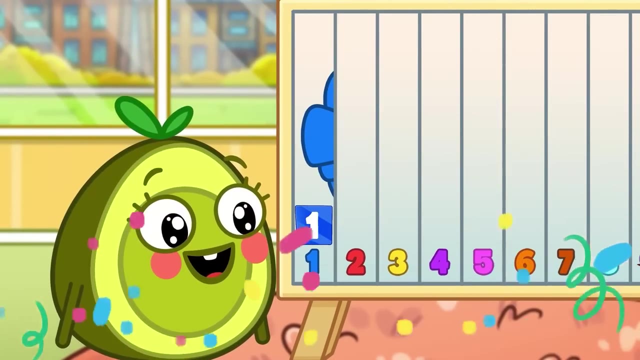 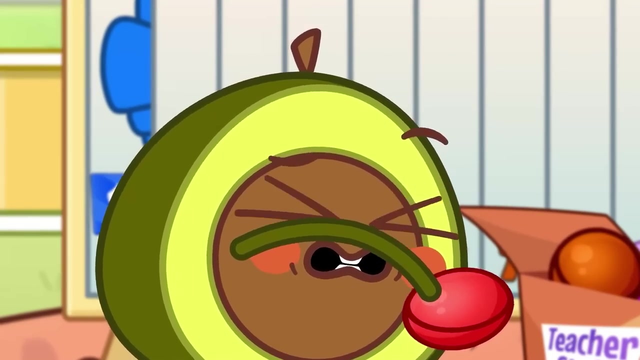 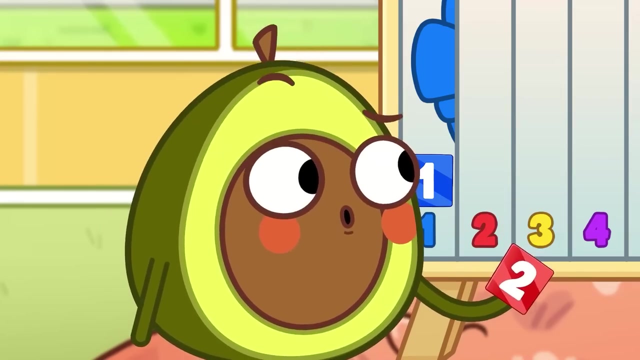 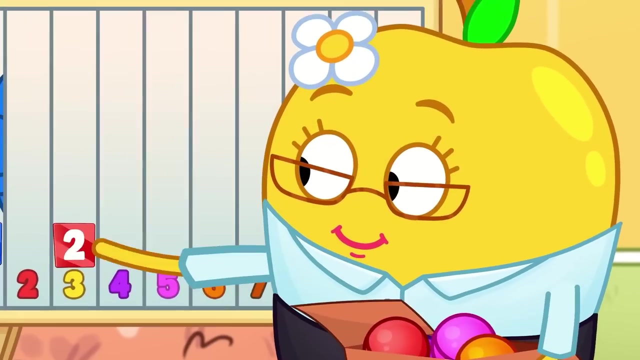 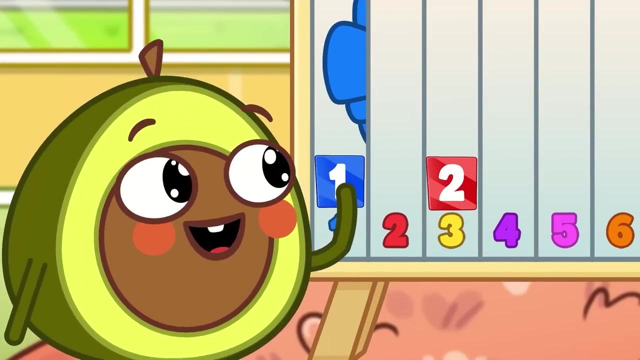 That's not right. Try again. Penny, Yes, One is the first number. Your turn Pit, It's number two. It doesn't go there. Oh, Remember, Two comes after one. That's right. One and then two. 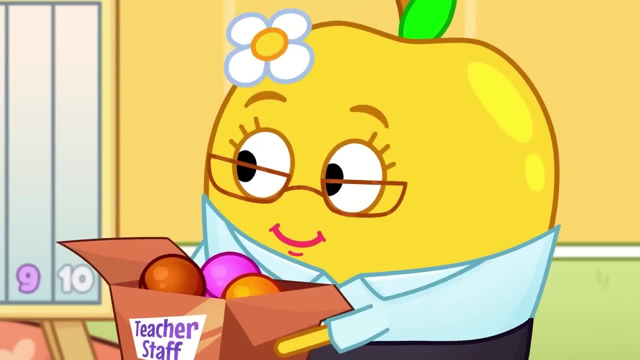 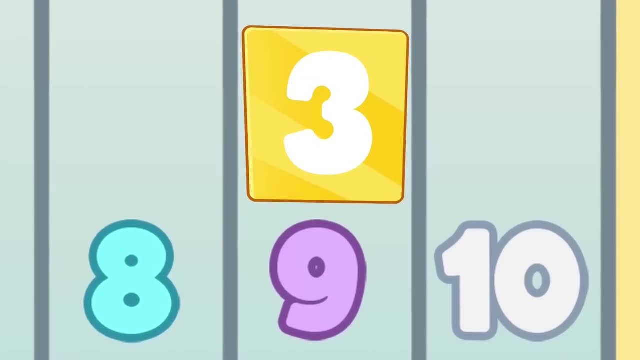 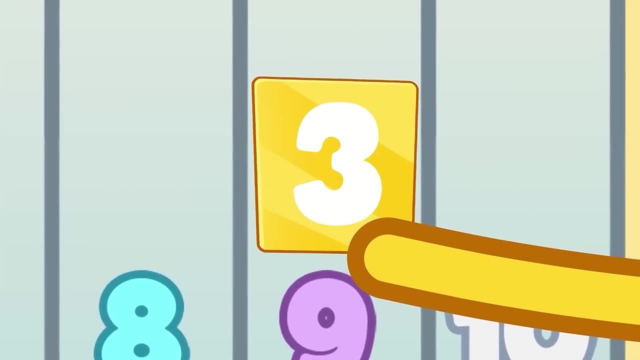 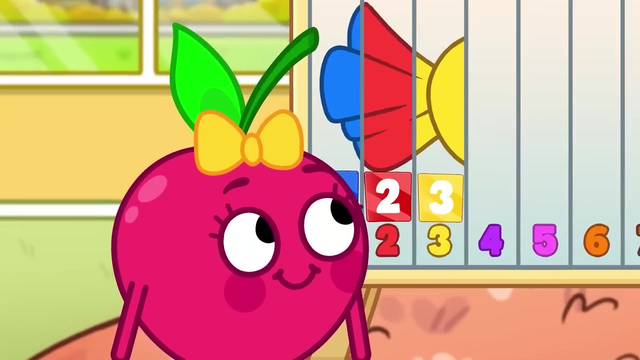 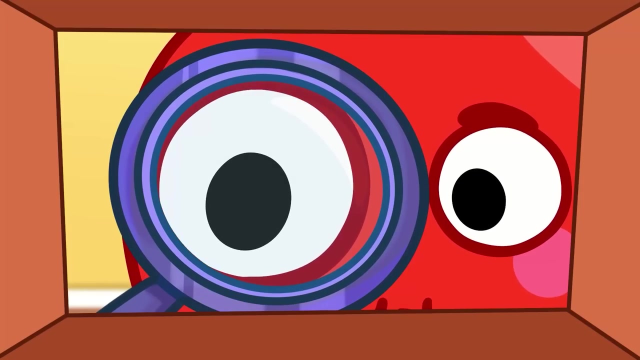 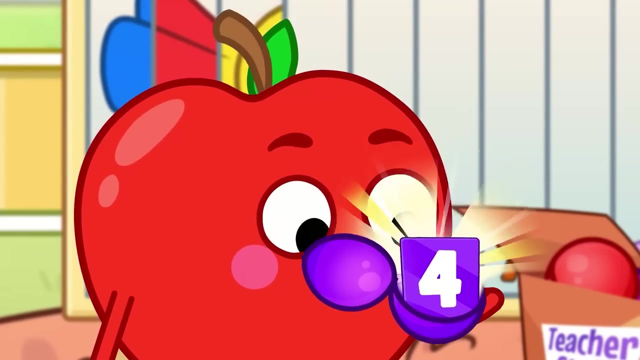 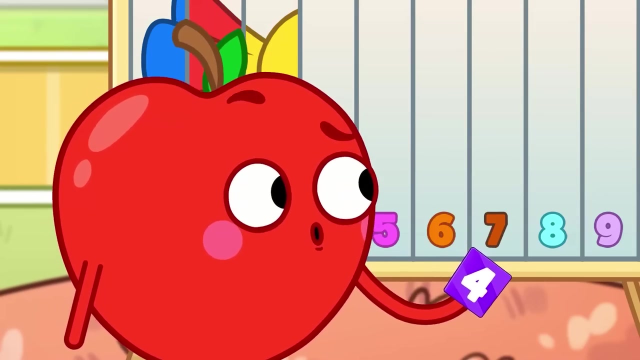 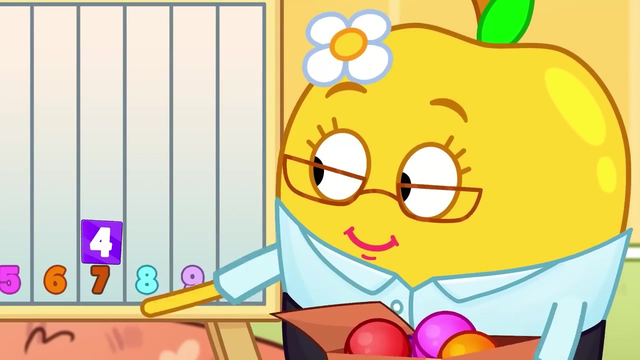 What number did Cherry pick? It's number three. Hmm, is that correct? That's right. One, two, then three. Apple, you try. It's number four. Four, Does four go there? Try putting it after three. 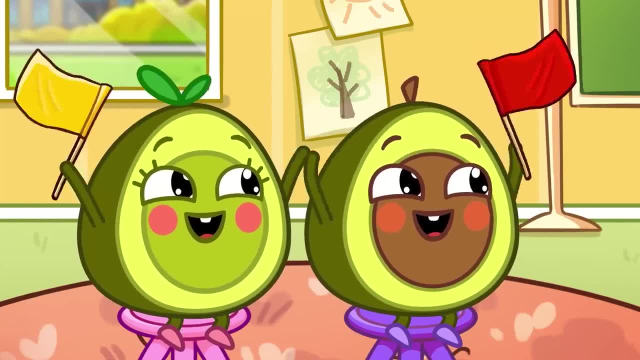 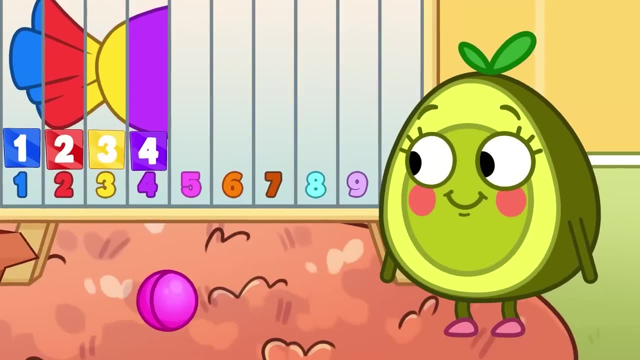 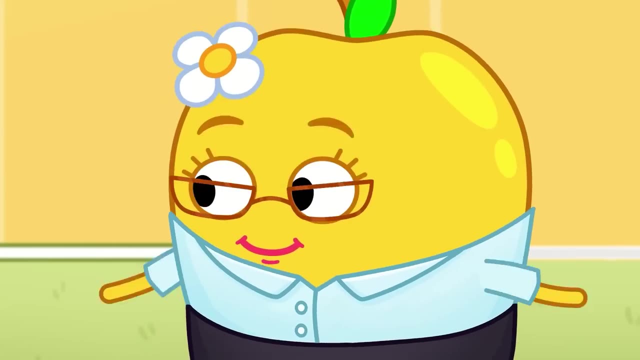 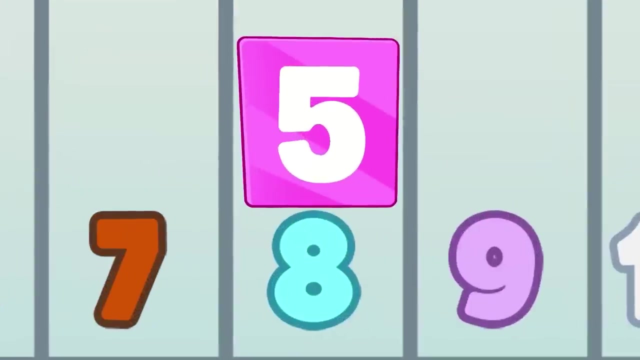 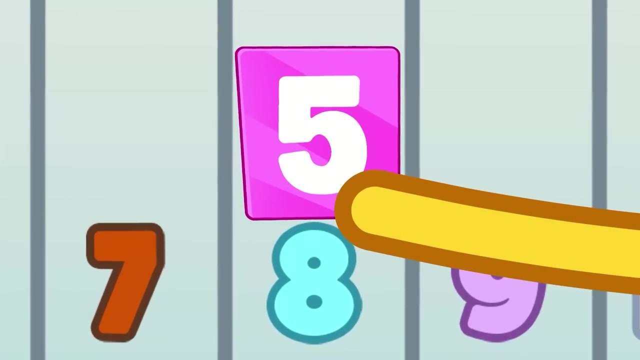 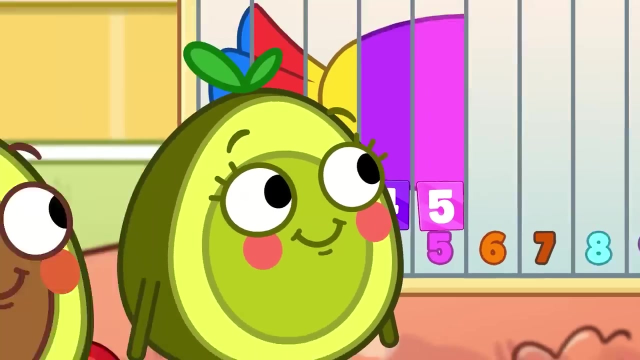 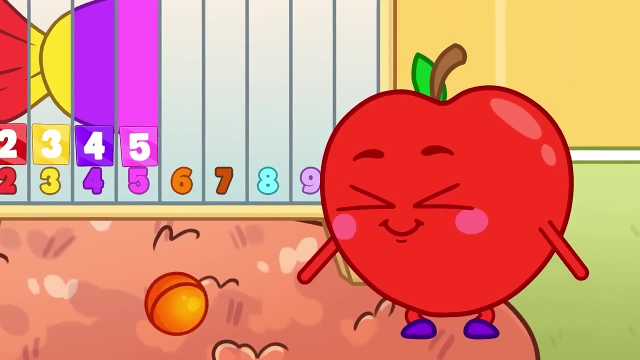 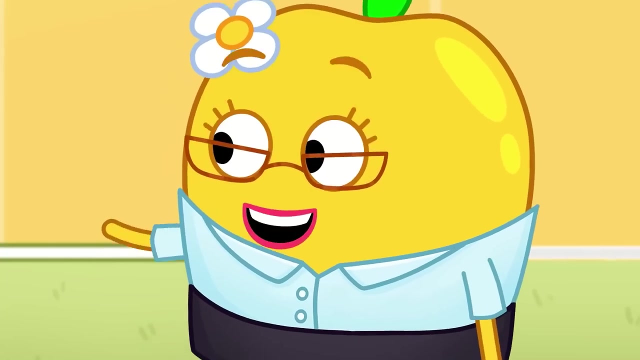 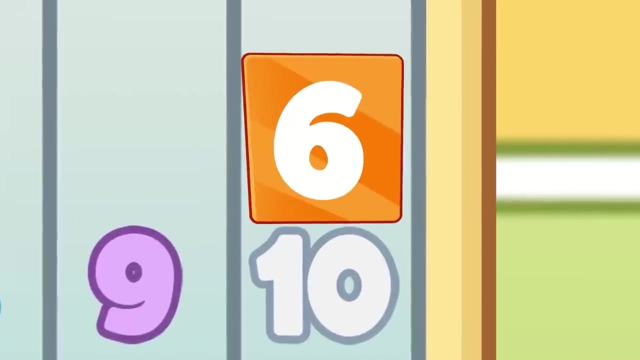 Hooray Pit's using his crab hands. Wow, There's so many. Wow, Penny will help. It's number five. That doesn't look right. Five follows four. It's the next number. It's number six. Is that the right spot? 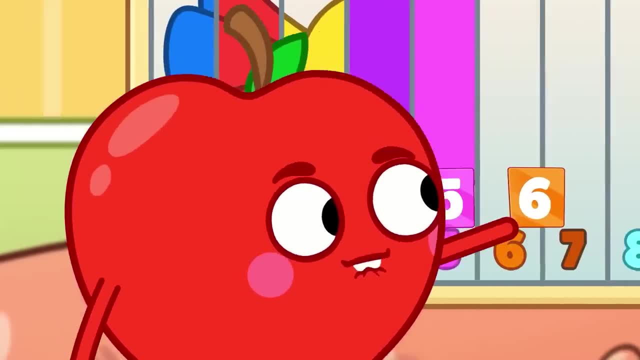 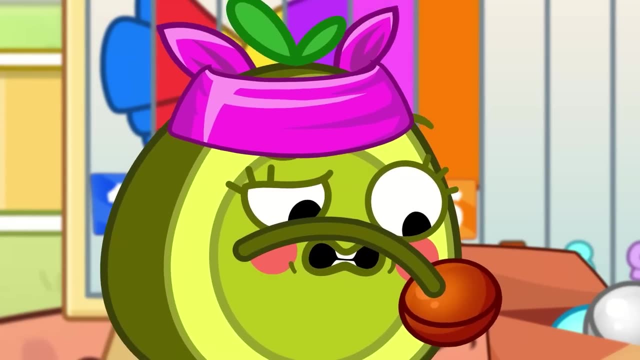 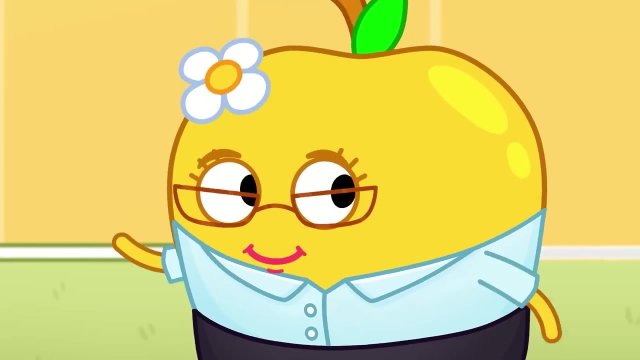 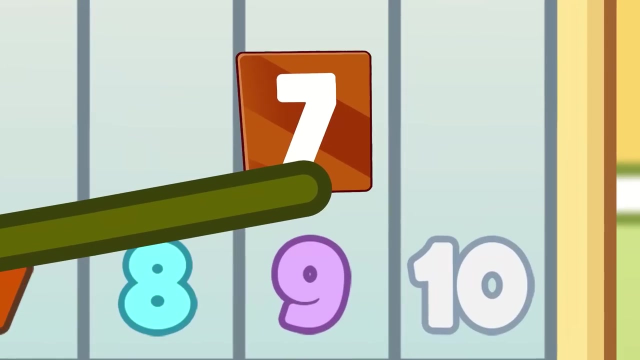 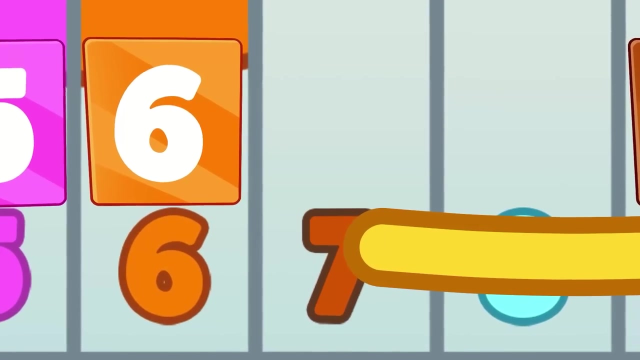 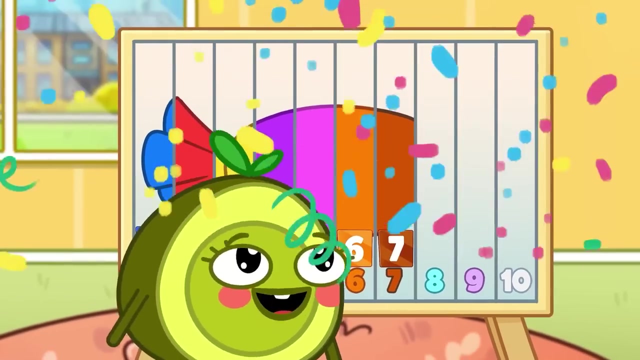 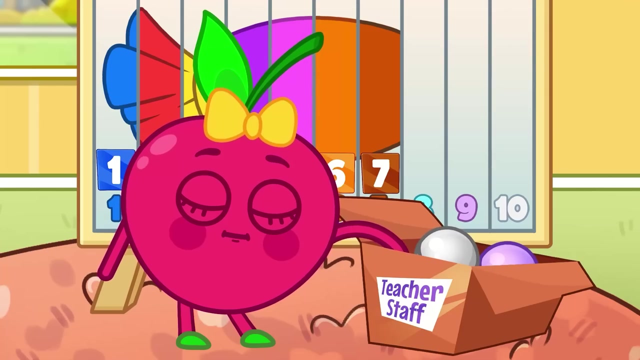 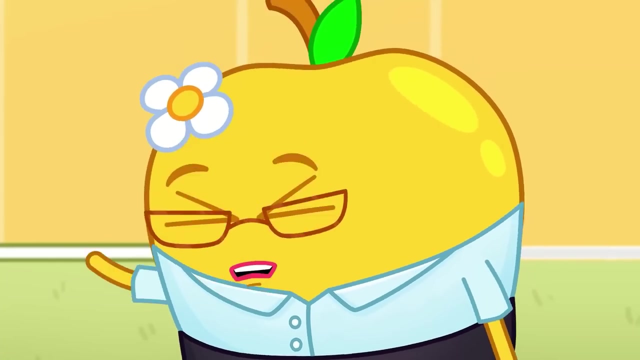 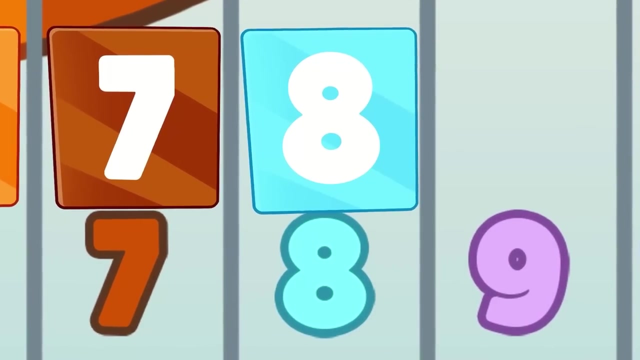 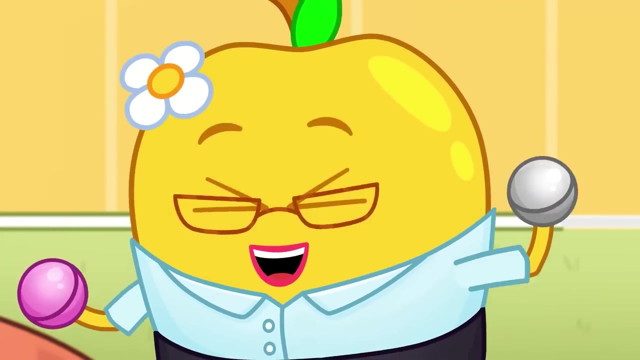 Six comes after five. Hey everybody, It's number seven. Where should we put it? Not there, Penny, It's number eight. It's your turn. It's number eight. That's the right spot. There are two numbers left. 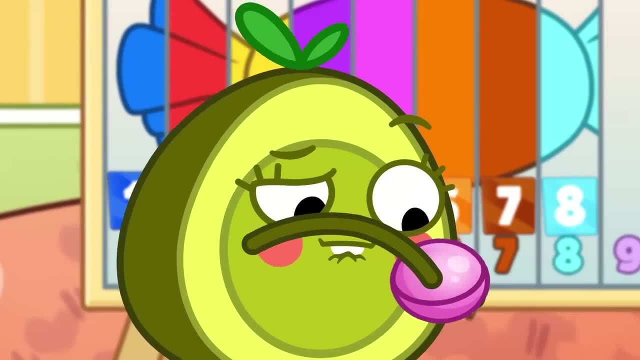 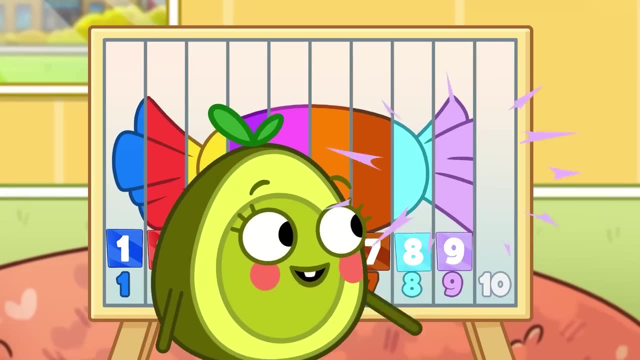 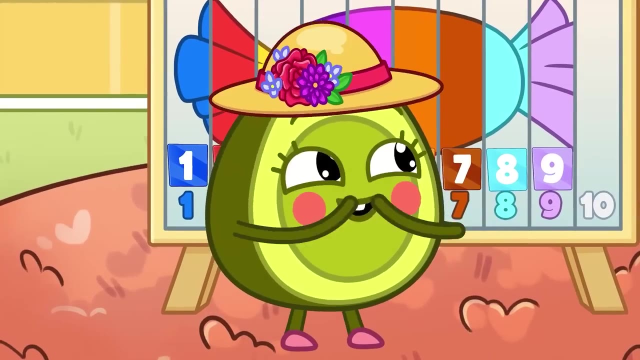 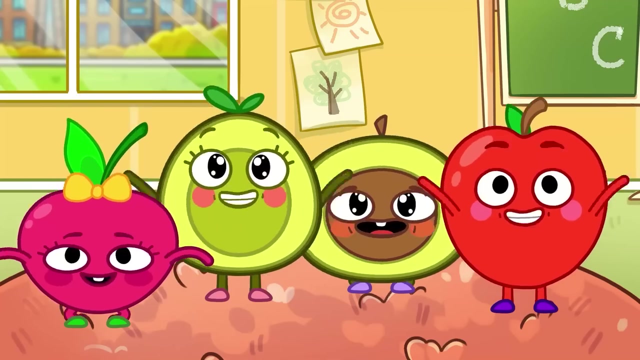 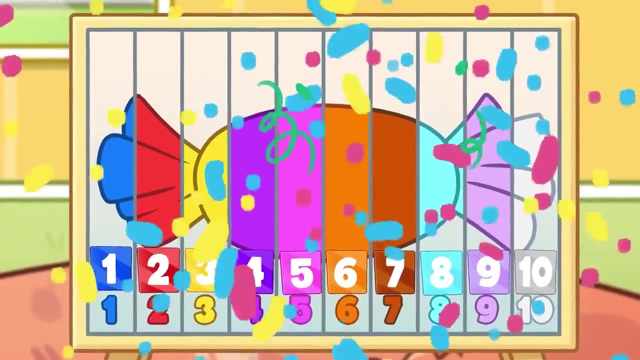 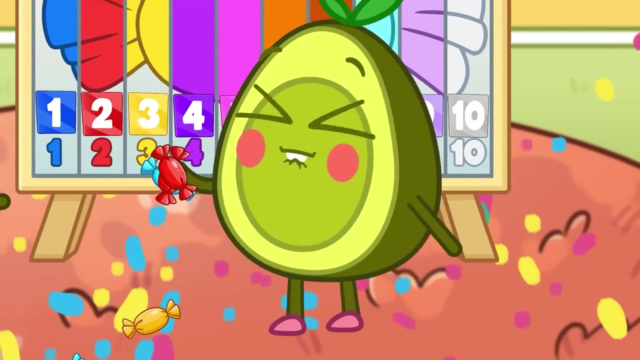 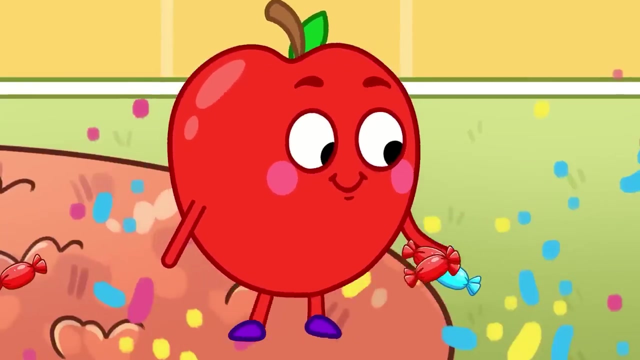 I'll have the pink one. It's number nine. What's the last number? It's number ten. It's number ten. The numbers make candy. Let's count them: One, two, three, four, five, six, seven, eight, nine, ten. 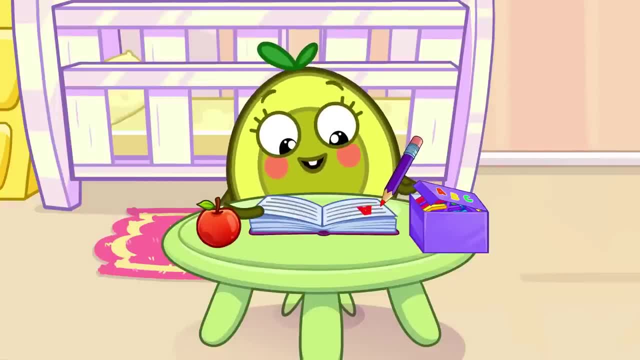 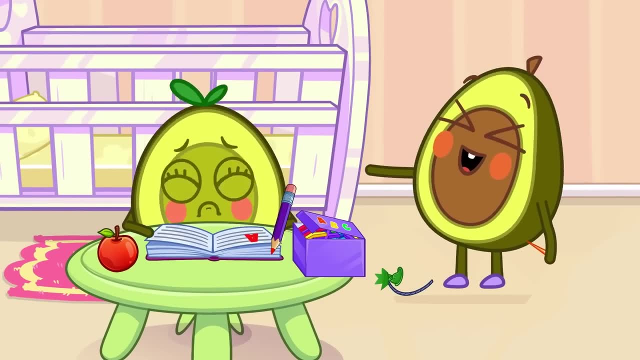 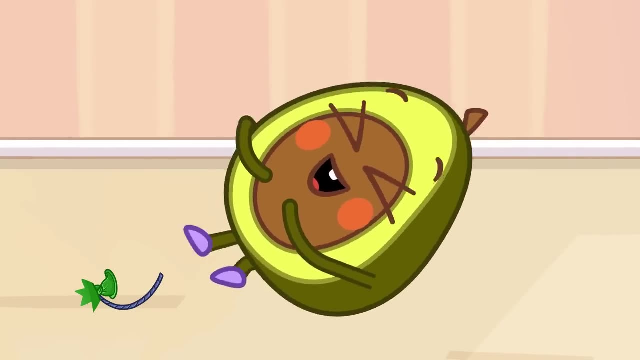 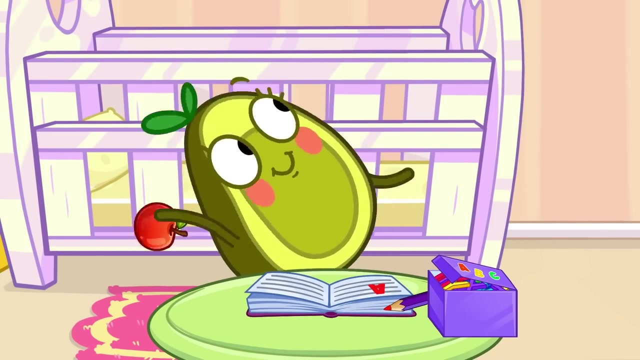 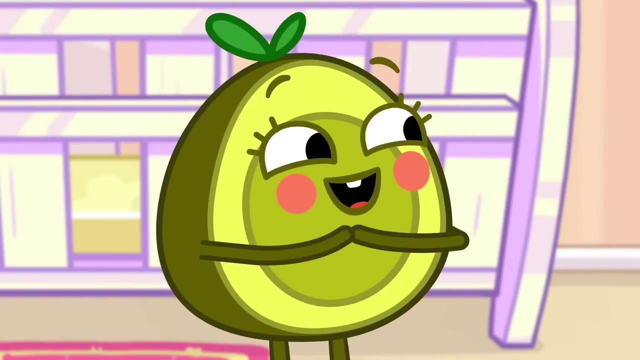 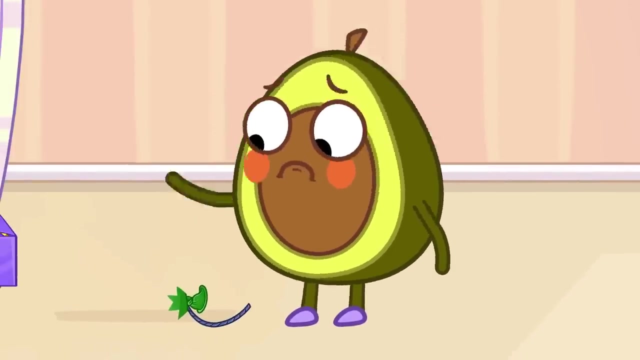 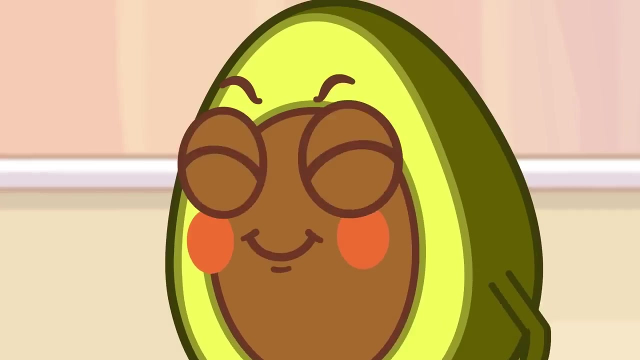 Penny is learning the alphabet. Penny is learning the alphabet. What is Pit up to Pit? you made Penny smudge her letter Apple. Apple starts with the letter A. Hit you popped your balloon. Hit wants an alphabet contest. Who will win? 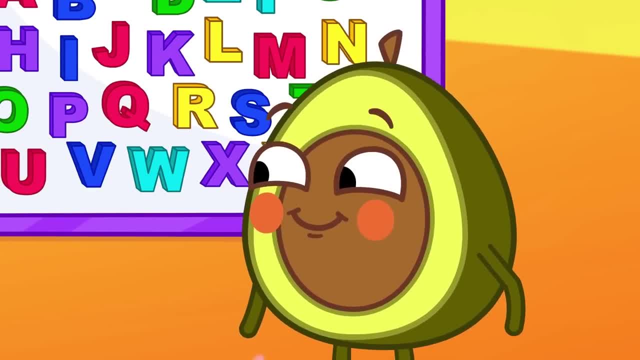 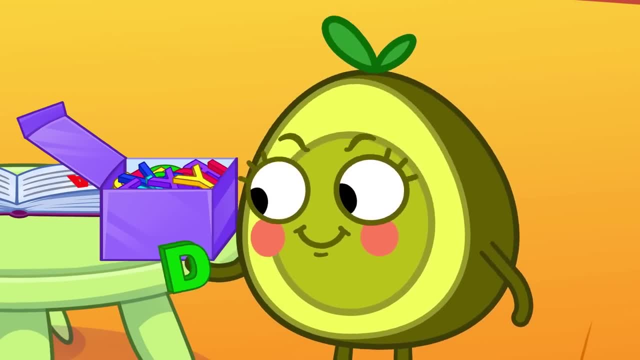 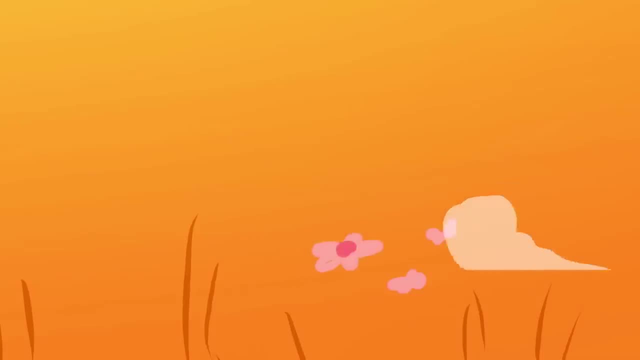 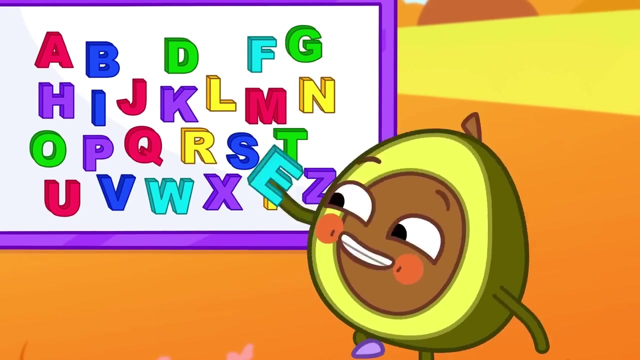 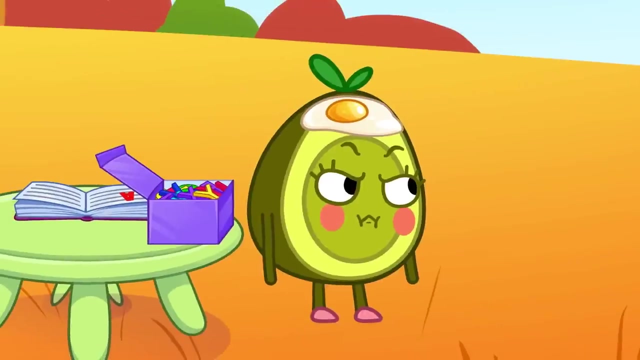 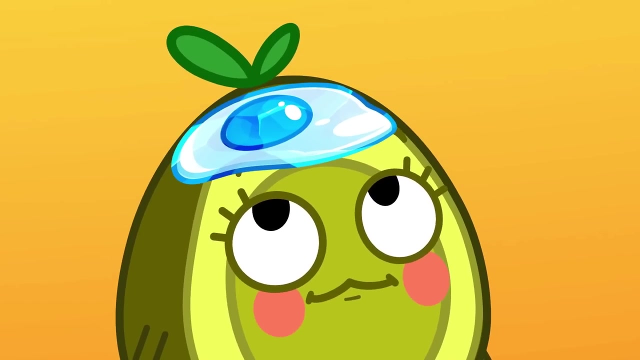 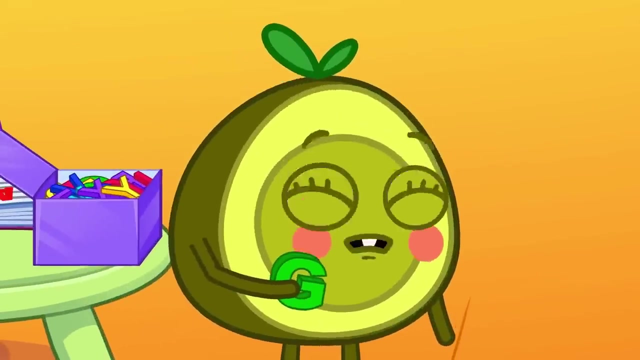 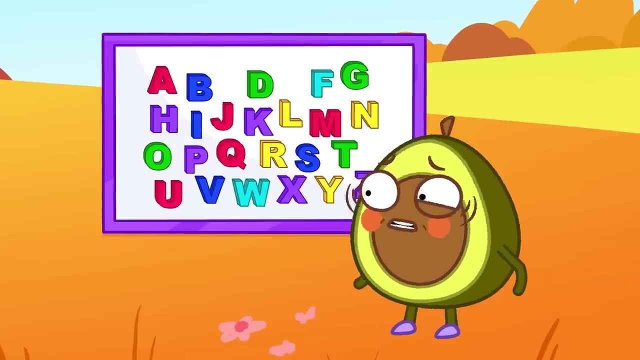 C- cat What starts with D and hates cats. Z- dog, Bye-bye kitty. That wasn't very nice. The egg landed on Penny's head. F- frost- Penny froze the egg. What letter is next? G- ghost Watch out Pit. 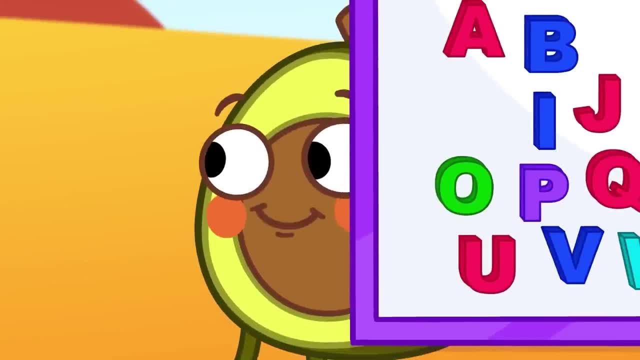 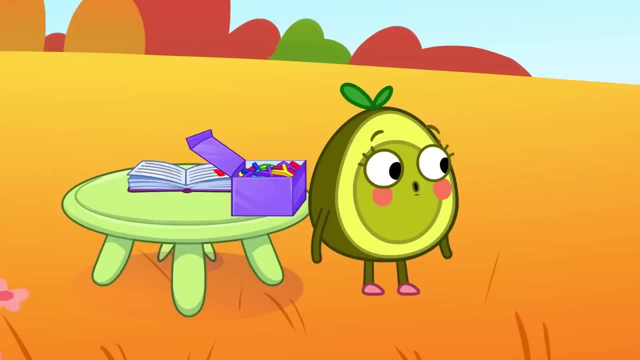 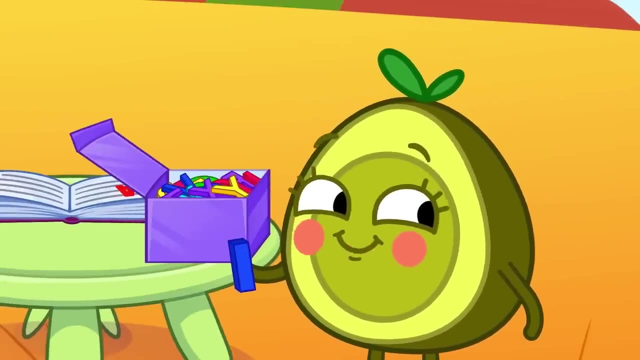 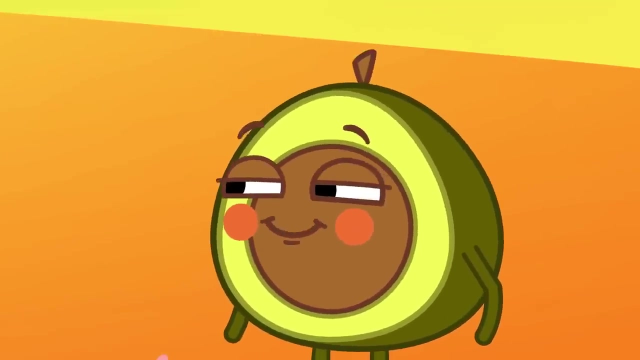 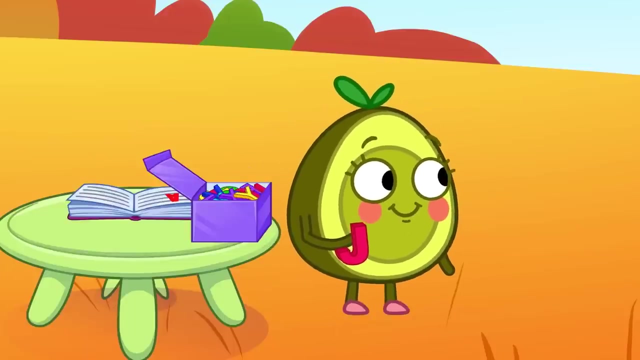 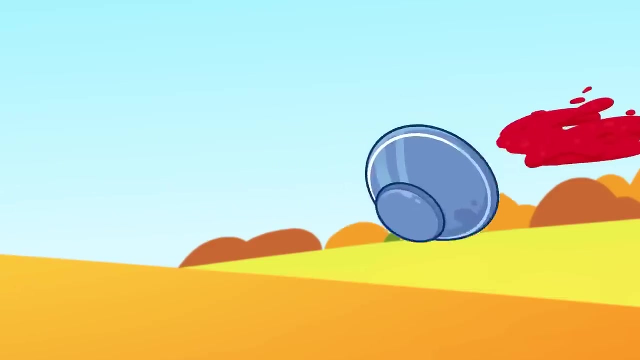 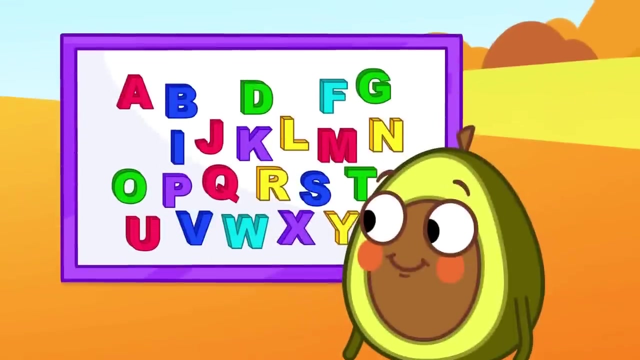 H helicopter, H helicopter. Wink, It'll blow that ghost away. I Ice cream. It loves ice cream. Try again. Penny J Jam Jam can be really messy. What's next? Pit K Key. 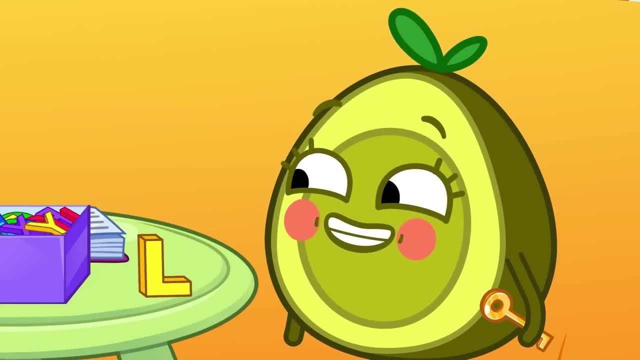 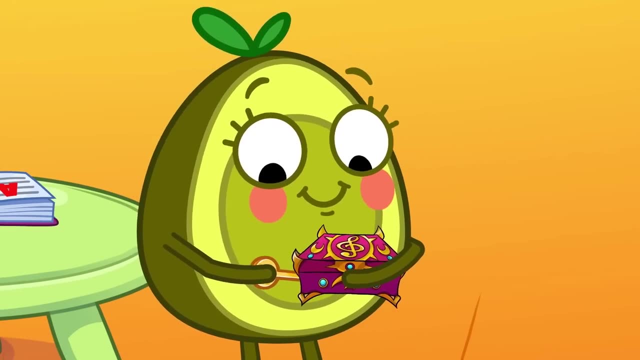 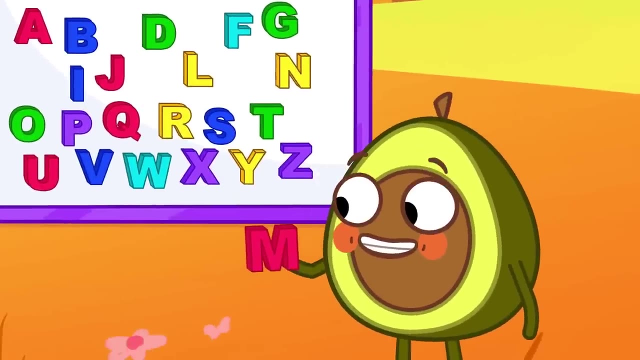 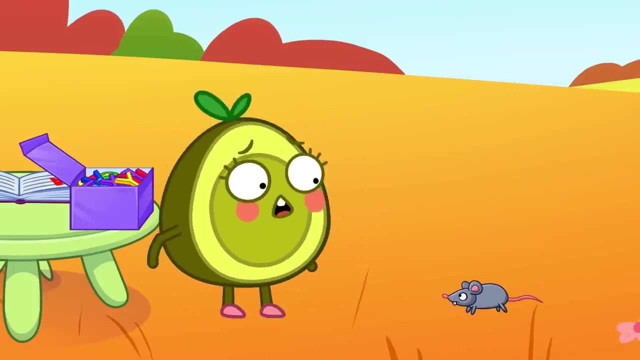 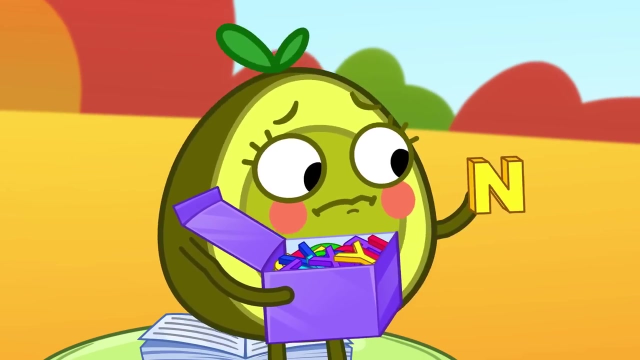 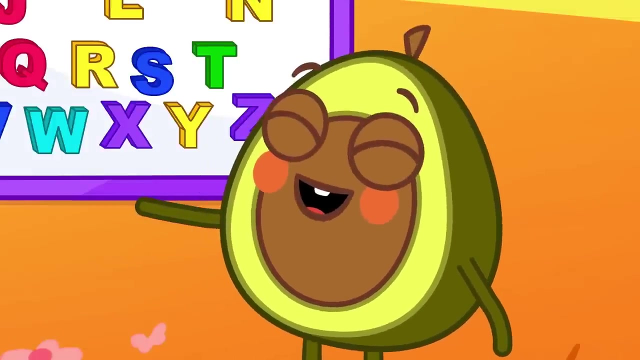 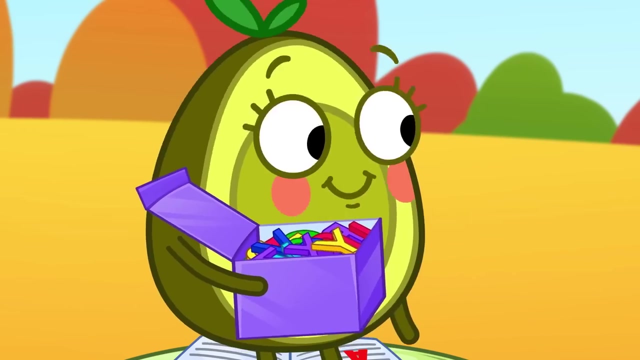 What does a key open? Ow A lock. It's a pretty music box, M Mouse. Penny doesn't like mice. What starts with N M Mouse. Try another one, Penny. O O, Uh-oh. 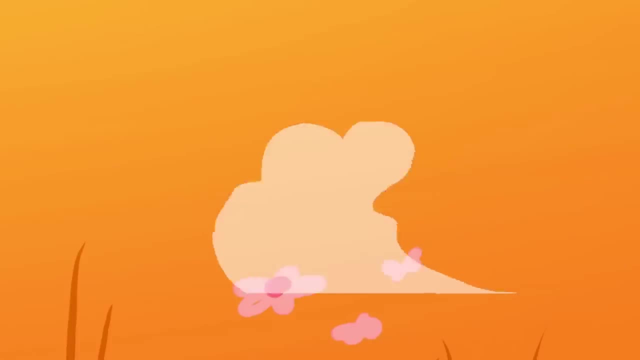 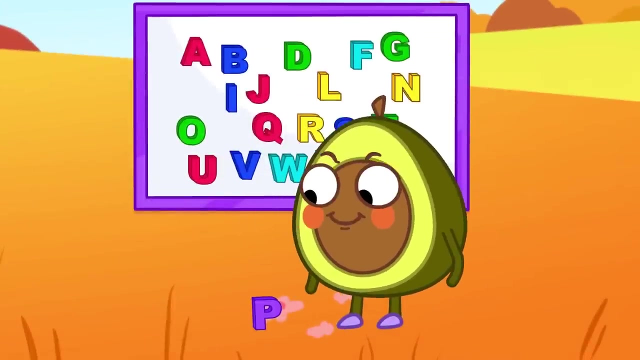 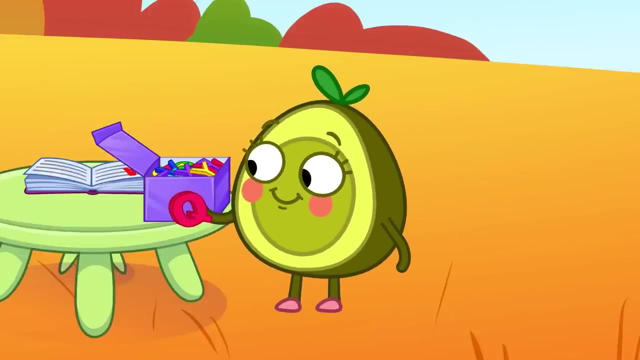 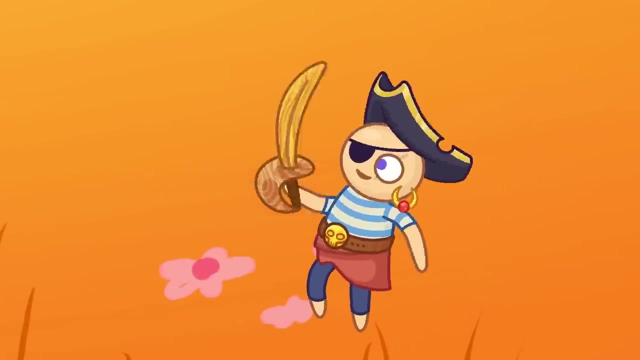 Mice don't like owls. P Pirate It O, O, O Q Queen. Now they can be friends. R Rainbow S Shark, The shark's back, M, M, M M. 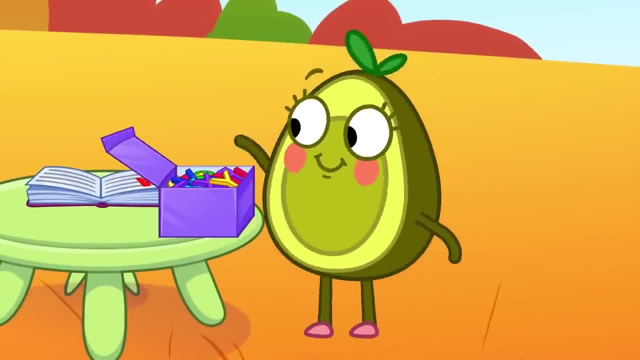 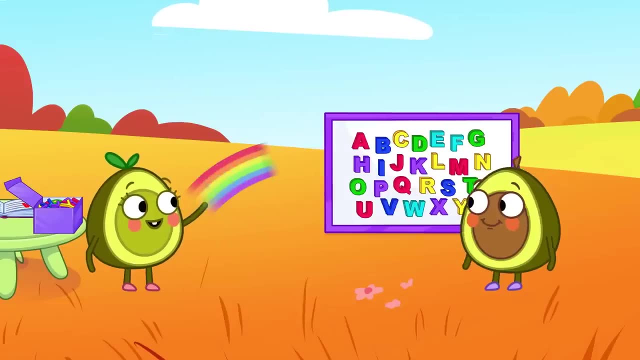 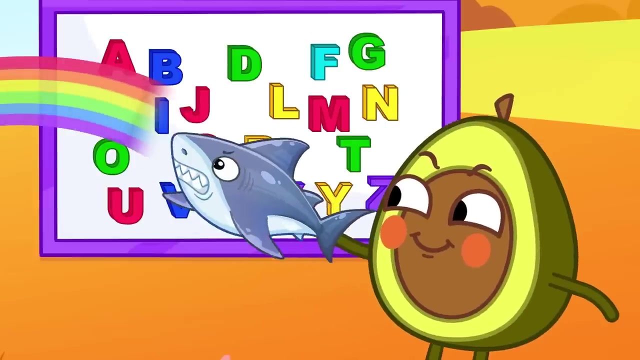 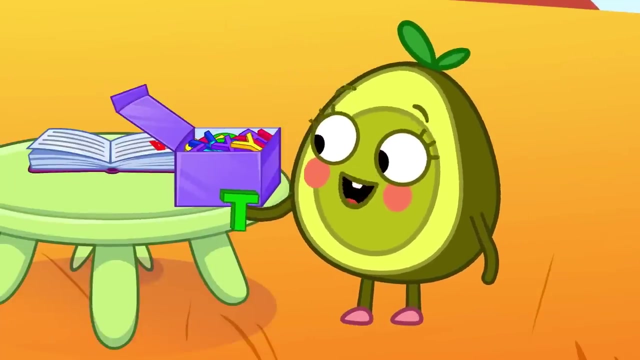 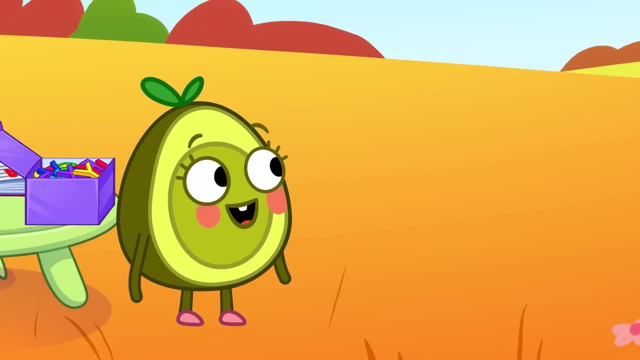 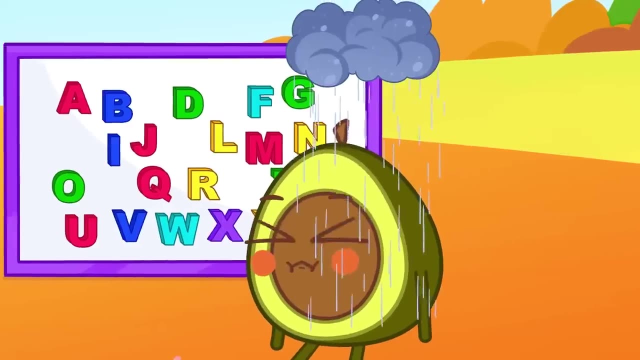 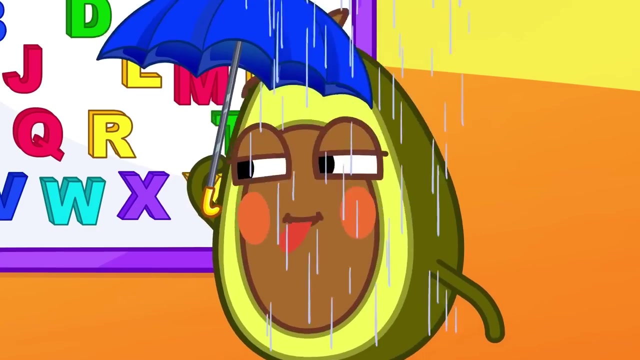 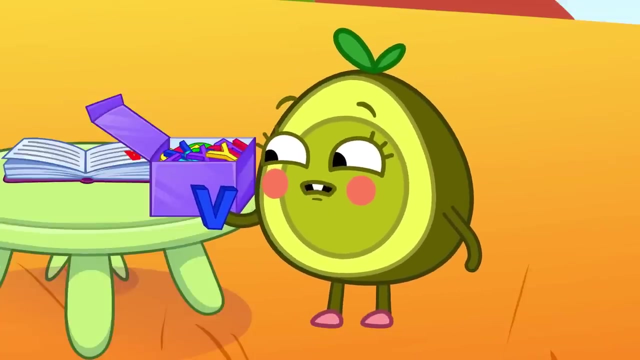 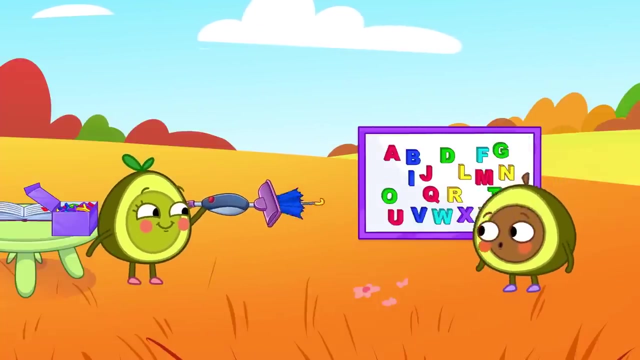 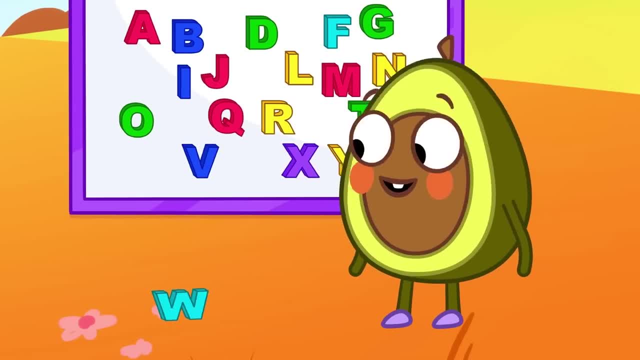 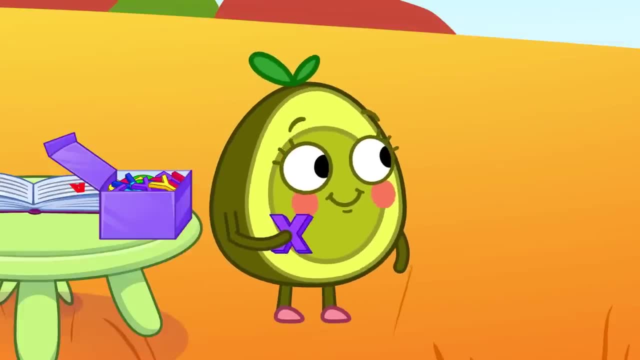 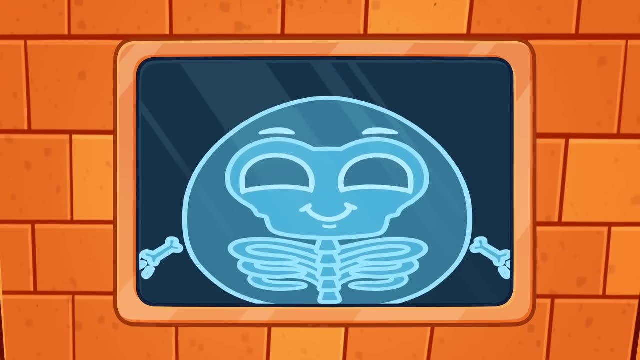 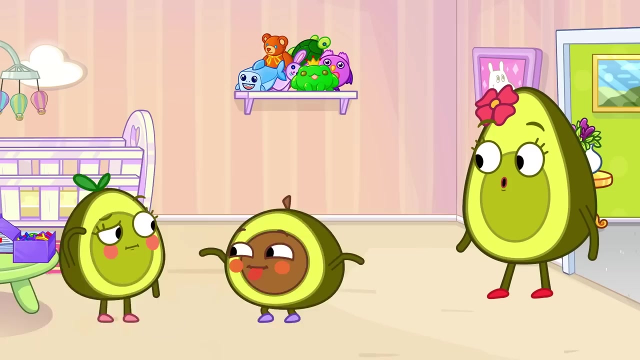 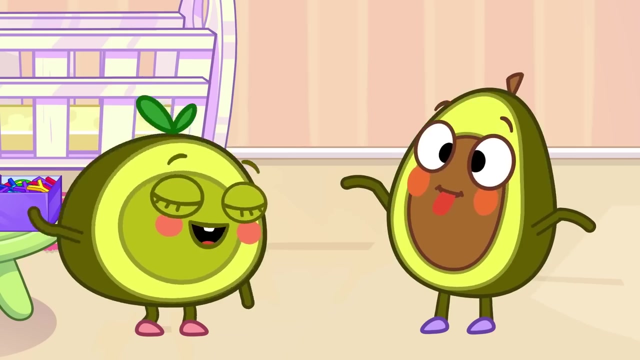 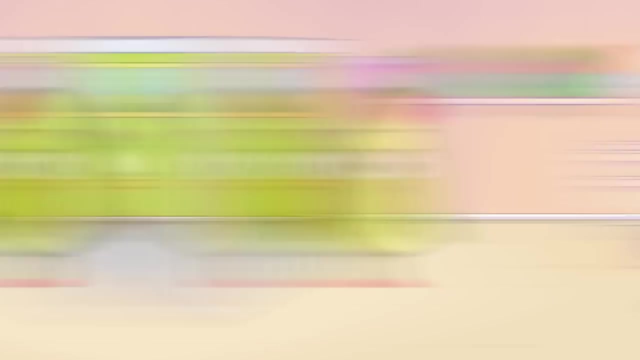 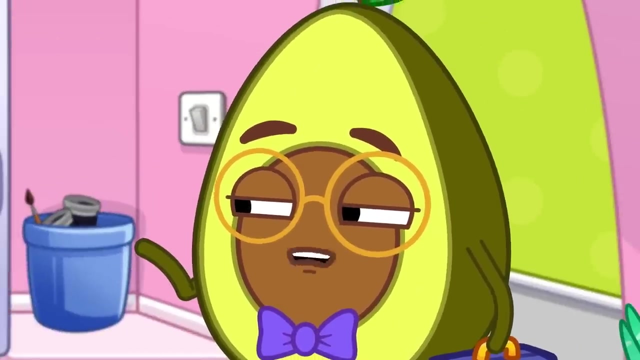 W Wall. To see through the wall, we need a X X-ray. Here comes Mommy. Do you want some yogurt? Y, Yogurt, Yes, Yogurt starts with Y. Are you ready to go to the zoo today? 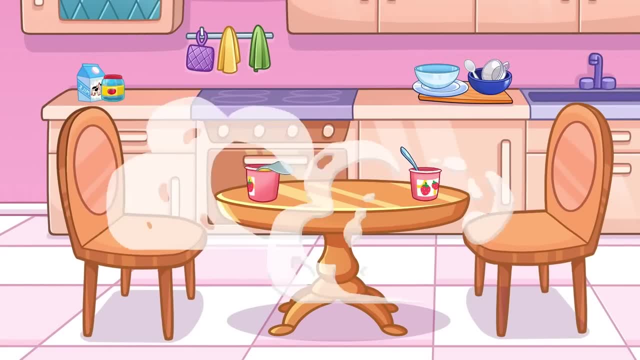 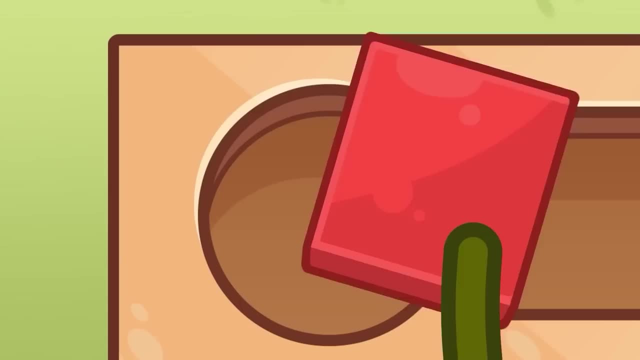 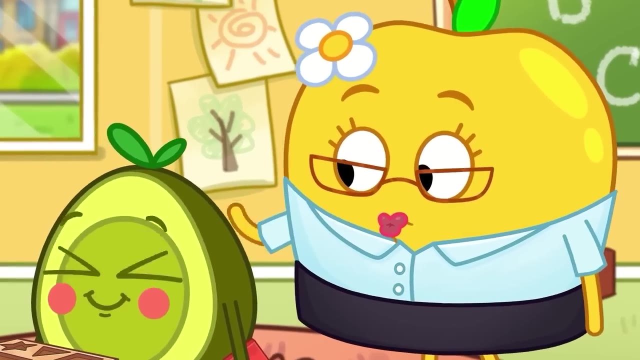 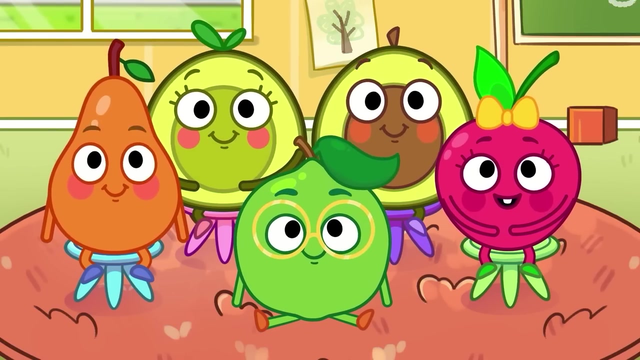 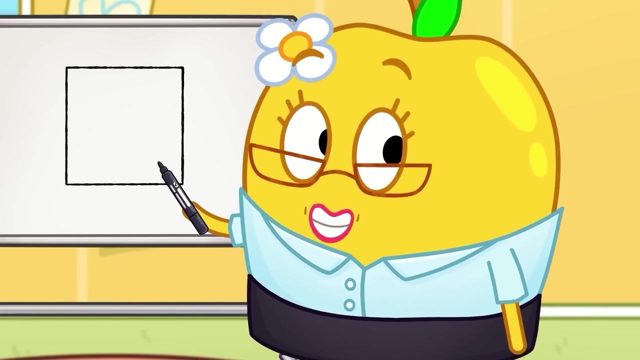 Dad, Zoo, Zoo. Have fun. Penny's having trouble with her shapes. Maybe Miss Apple can help Kids. let's play an interesting game. It's a square. Let's look for squares in this room. Penny's block is square. 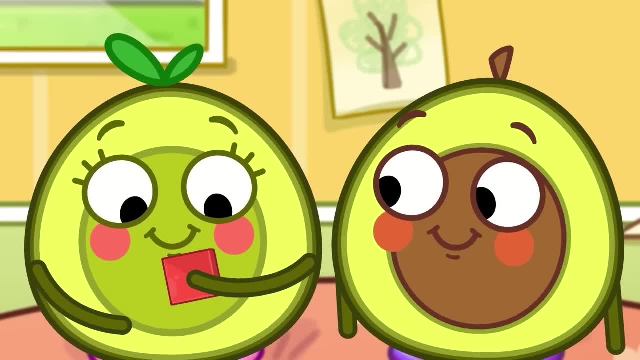 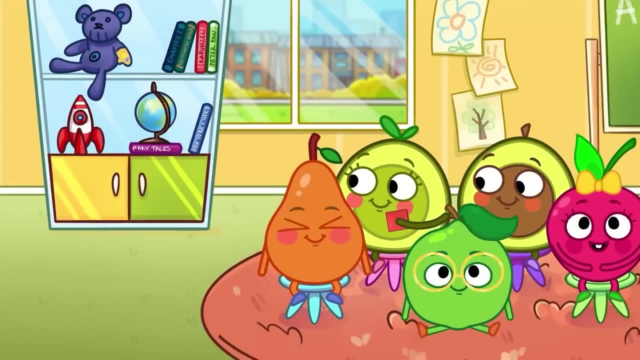 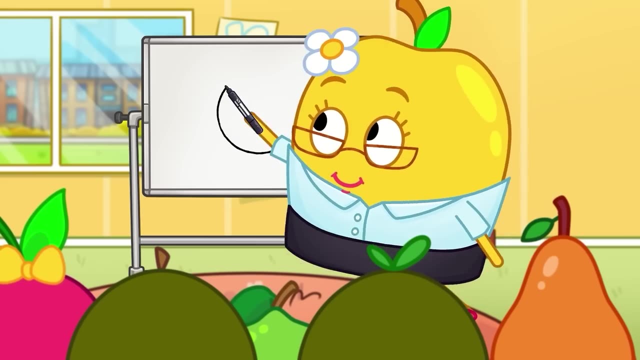 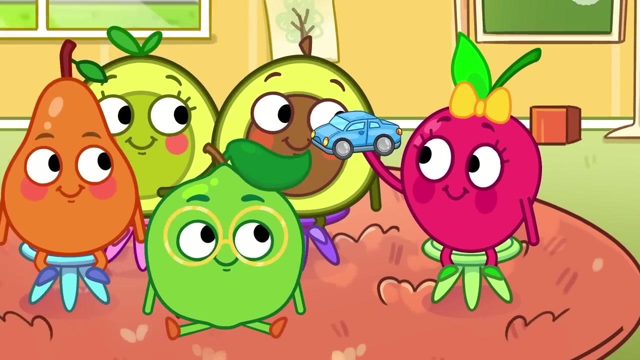 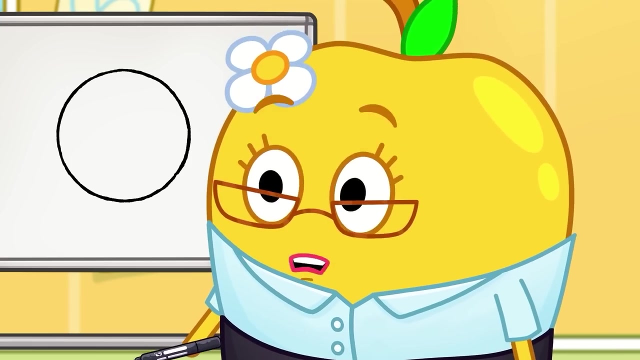 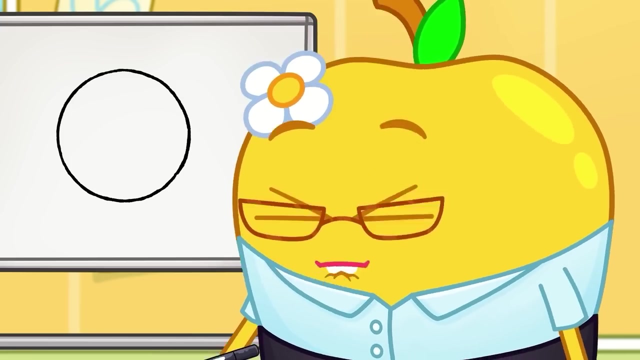 Right, Two more squares. Those doors are square, Well done. What's this shape? It's a circle. Car wheels are circles, Exactly A circle. What about a globe? It's a good example of a circle, A circle. 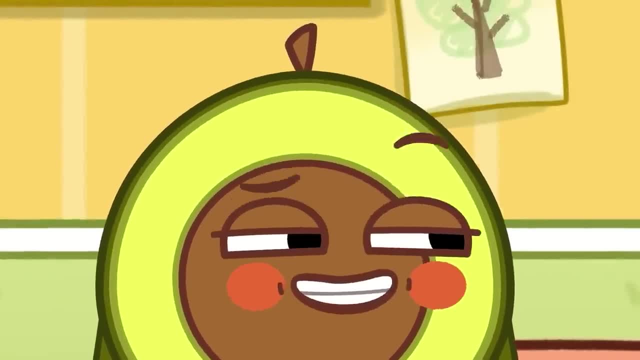 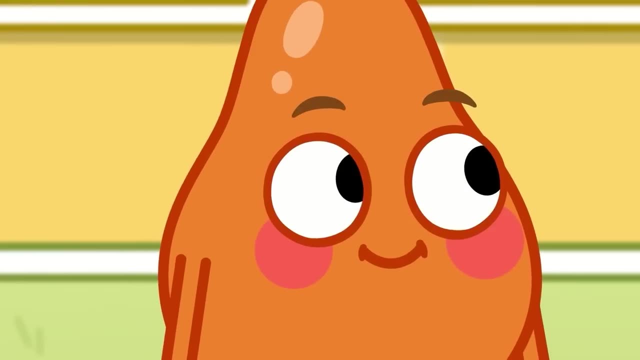 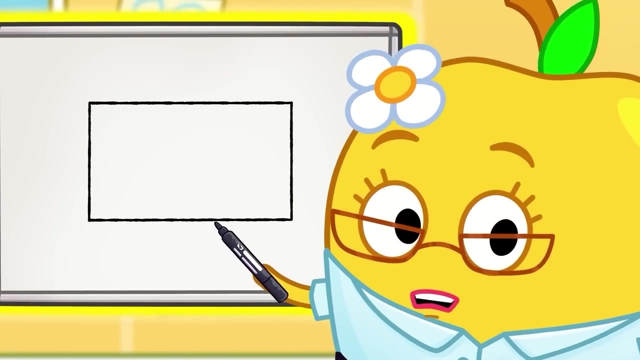 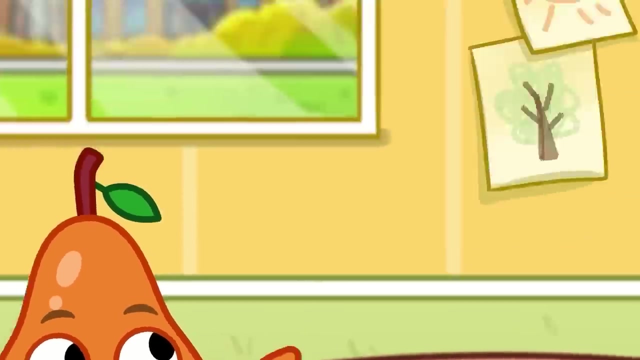 It's a square And a losphere. They're circles. They're circles And cherries are circle. It's very nice circle. I love circles. Hmm, What is THIS shape? It's a rectangle. So special… It's a rectangle. 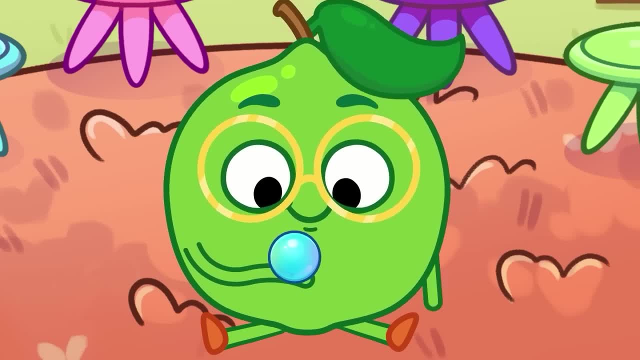 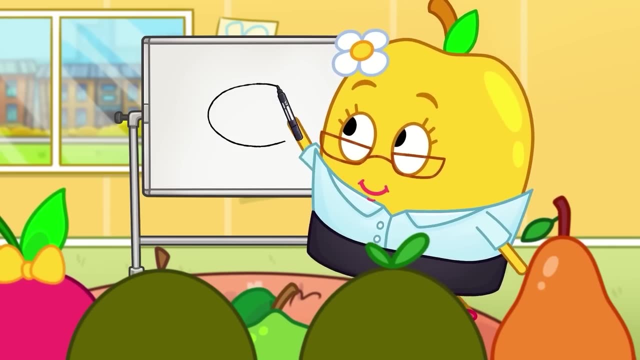 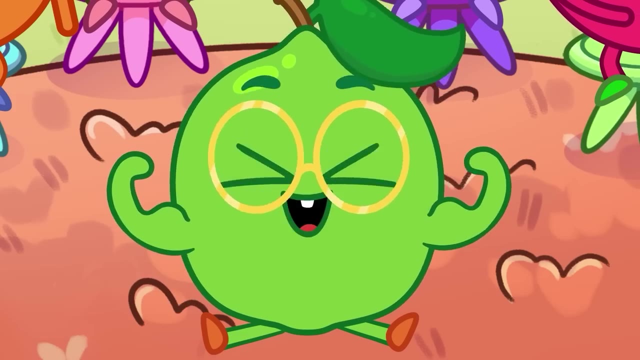 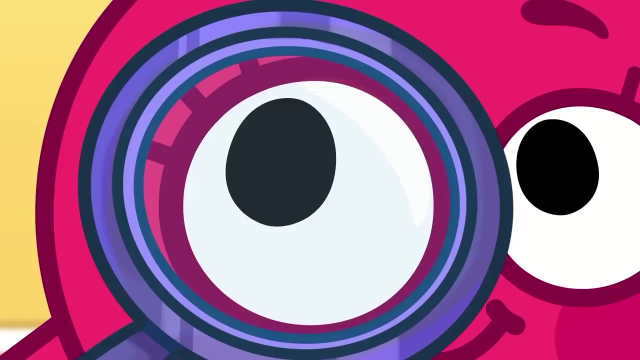 Great, We're going to check that again. Hooray, I do love Penthouse, So here we go. Look, I've flattened the circle And gotten you figure, an oval. Let's find some ovals. There's one. 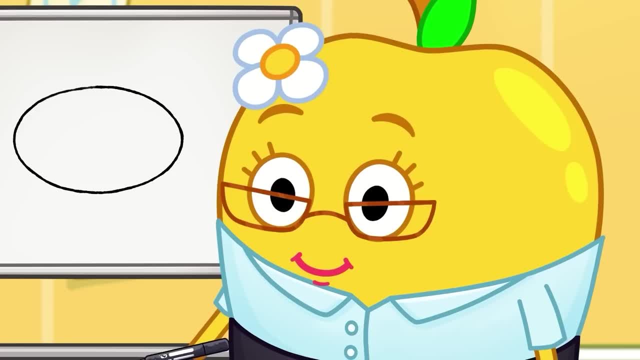 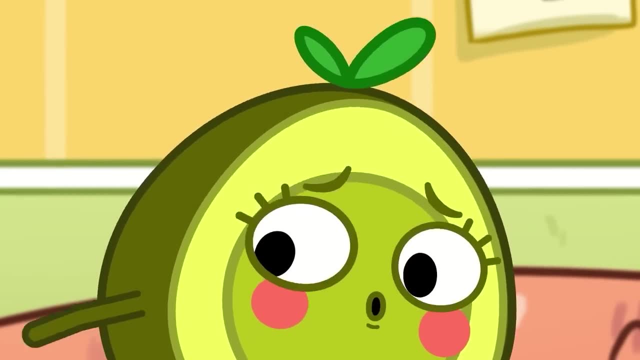 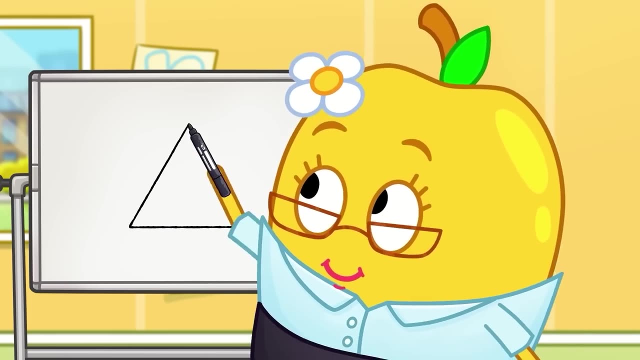 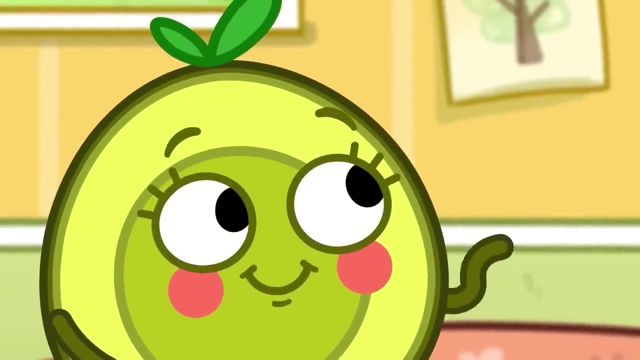 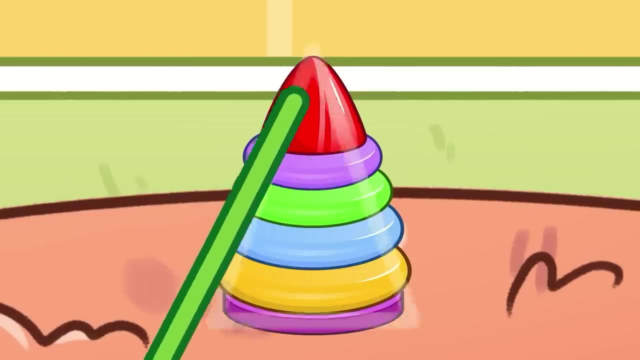 I have found an oval. Yes, What's wrong? kids, There are no more ovals in this room. And what's that? The rug is an oval, It's a triangle, The banner has triangles And the toy is like a triangle. 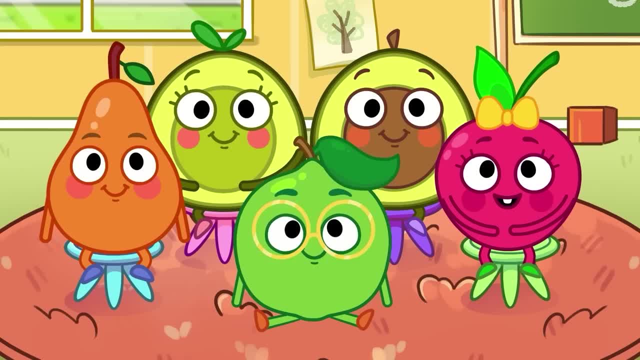 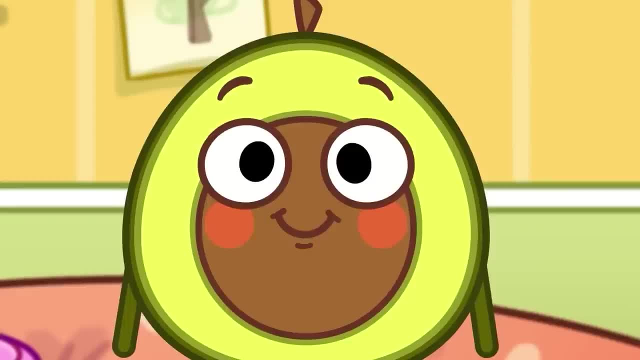 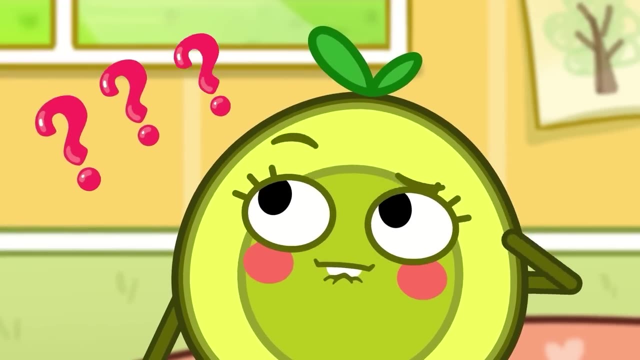 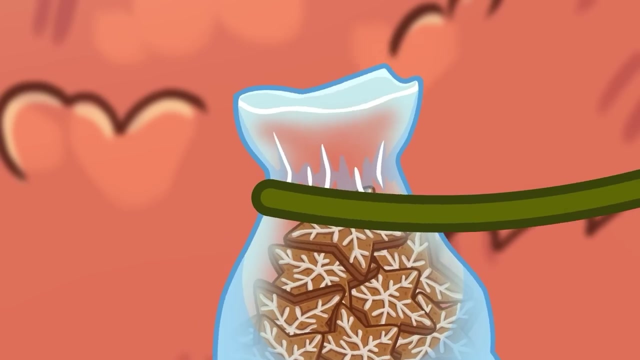 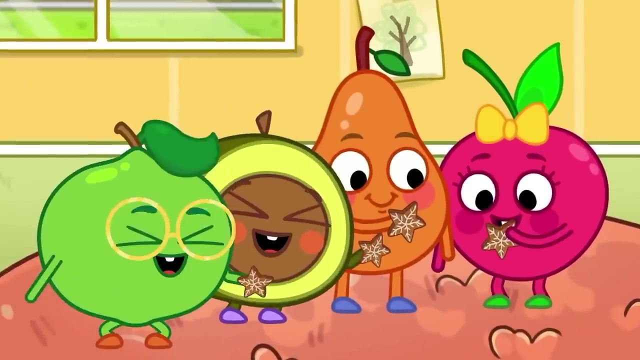 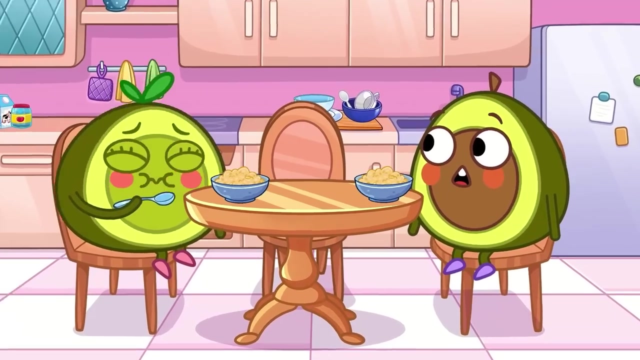 And now the hottest part, It's a star. Are there any stars? Penny will find some Yummy star-shaped cookies. Now, you know lots of shapes. Pit and Penny are having porridge for breakfast. Pit would rather eat chocolate. 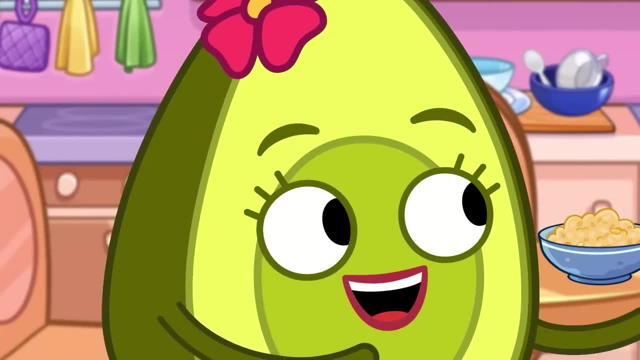 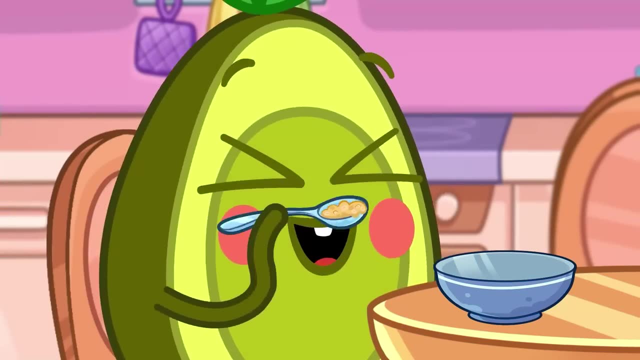 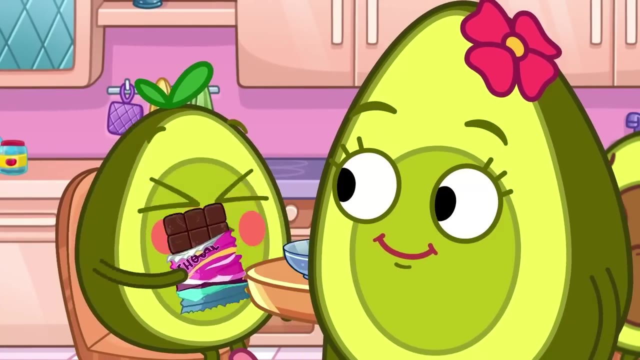 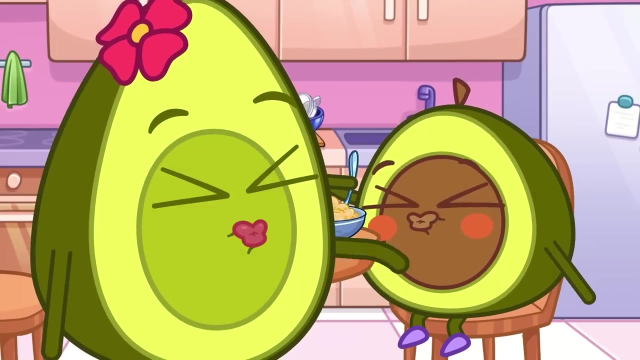 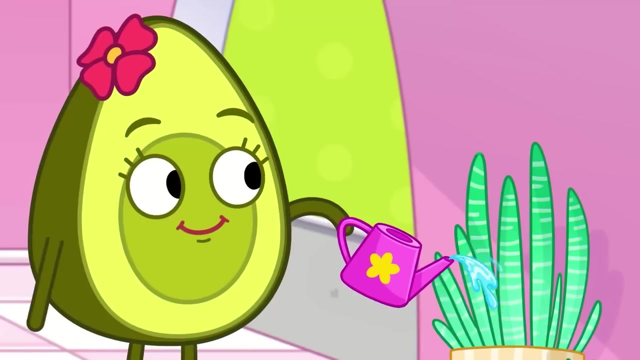 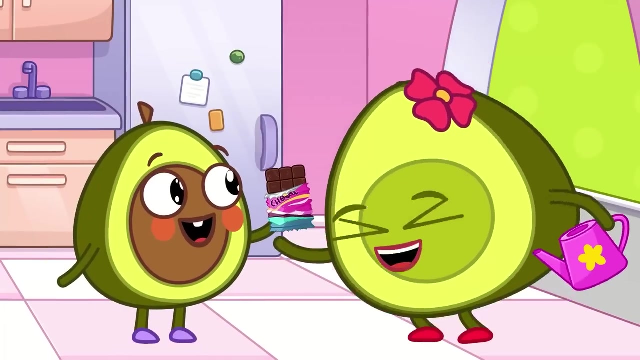 Eating sweets on the empty stomach is bad. Maybe you can have it later. Pit Oh Oh. Oh, Let's play a game. Hi-oh, Let's, let's go. tasty, Those foods are delicious. ấn Out� Innokipot. 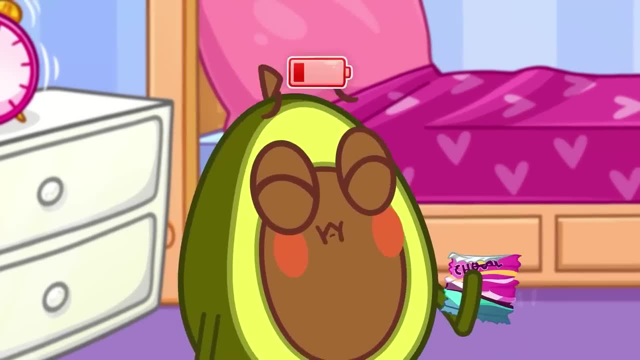 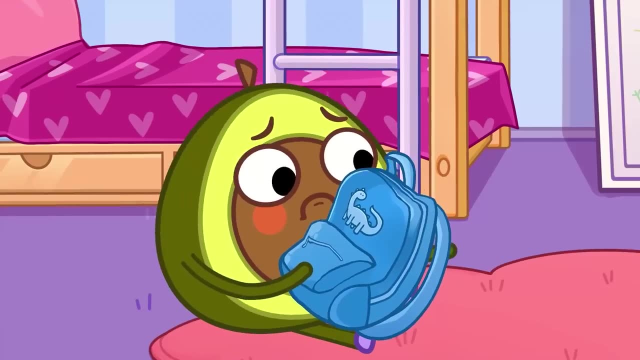 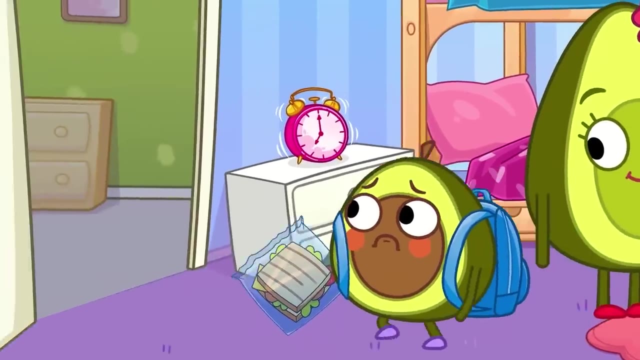 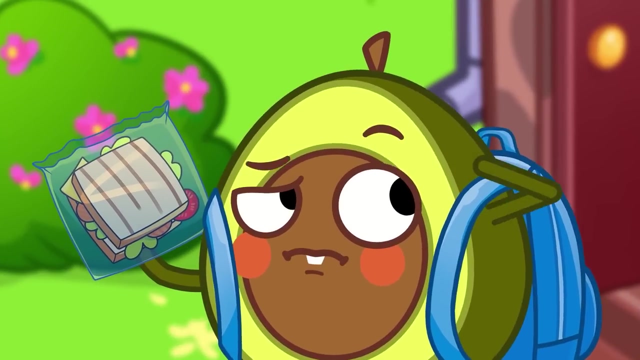 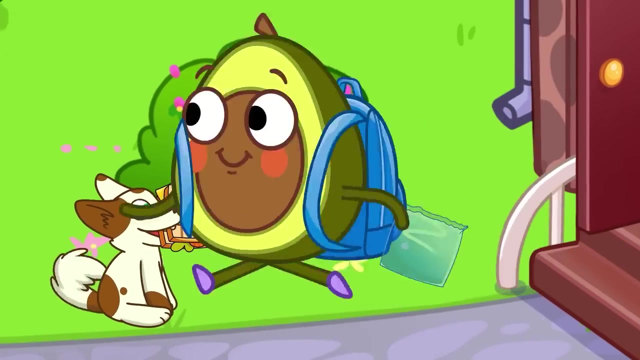 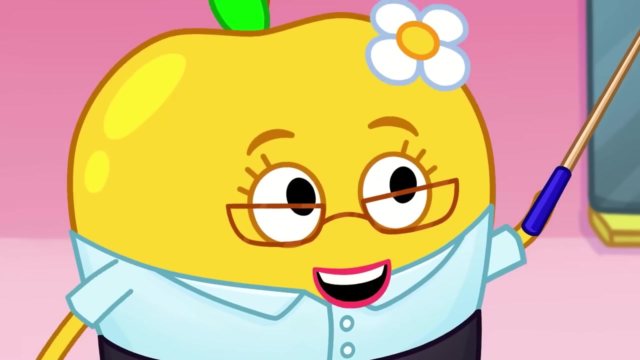 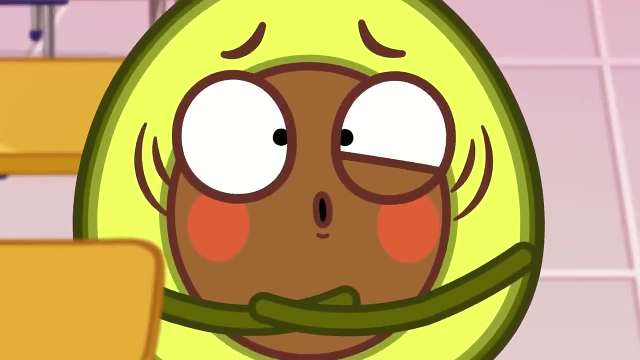 But Pit, chocolate won't give you energy. Yum Some healthy sandwiches for lunch. Pit will have nothing to eat later. And now he's so hungry. Pit, what letter is this? He's too hungry to think, Uh-oh. 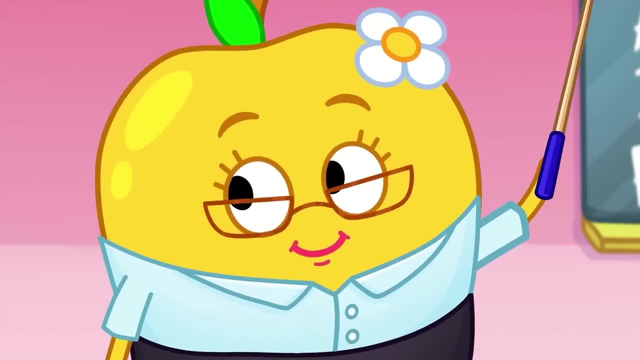 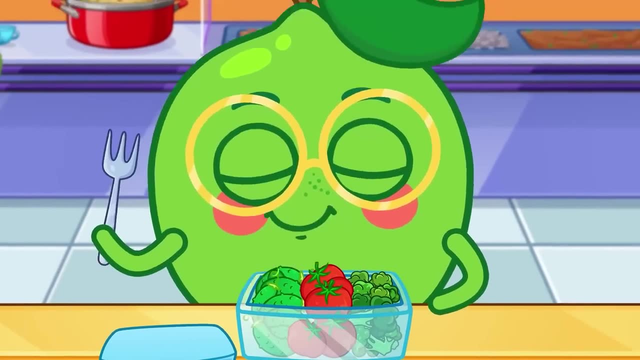 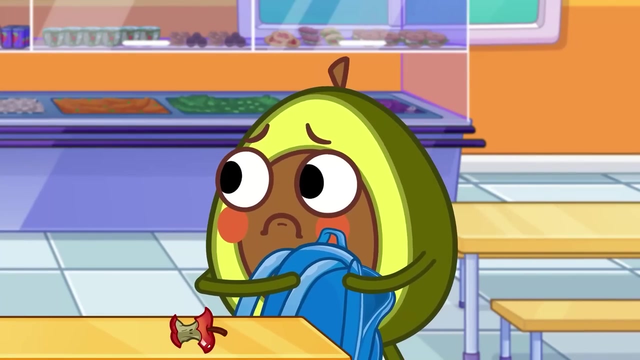 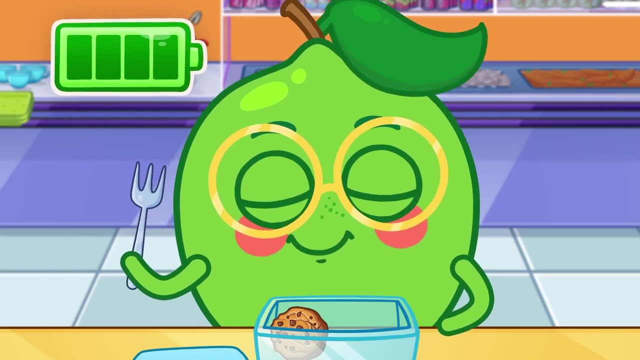 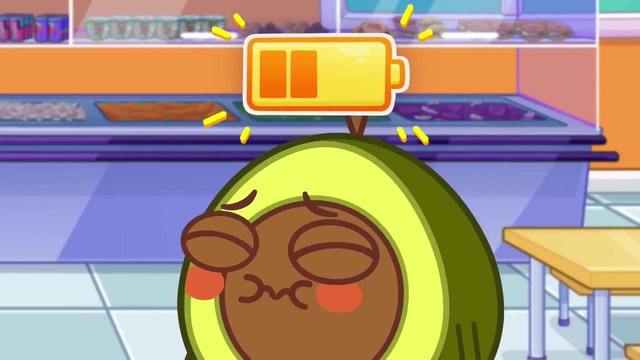 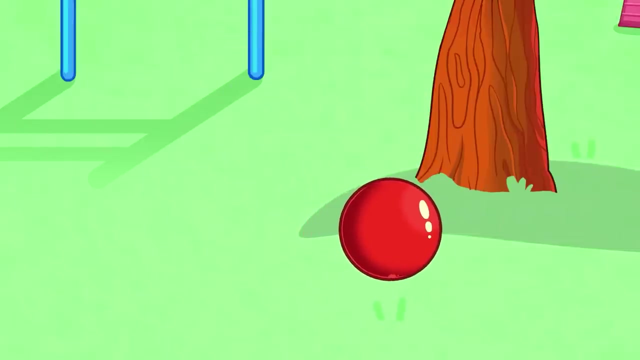 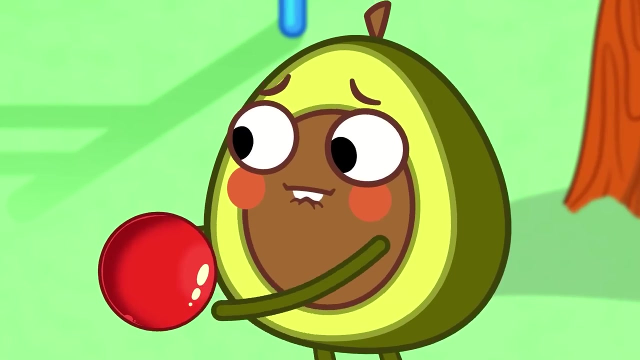 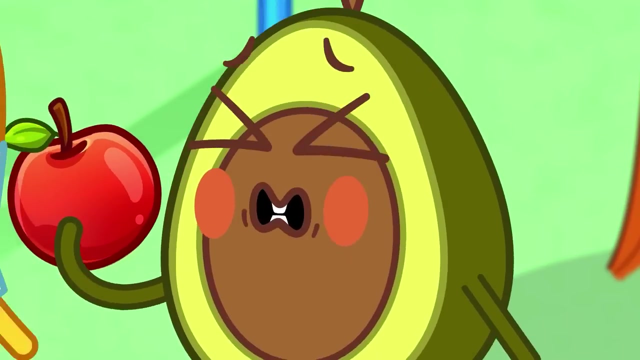 It's an A Yay, It's lunchtime. What will Pit eat? Penny has a sandwich. Lime has a salad. Lime gave Pit his cookie. Good, throw Lime. Is that an apple? Oh, Uh-oh, Sorry, Pit, It's just a red ball. 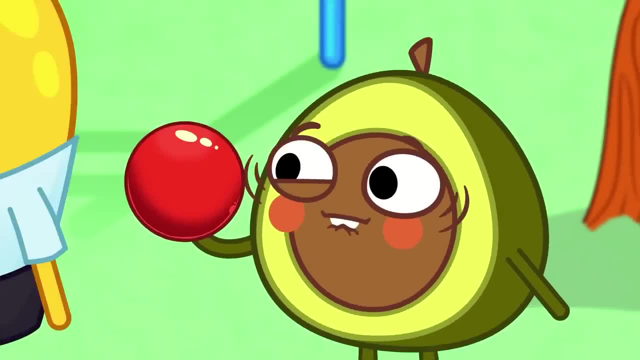 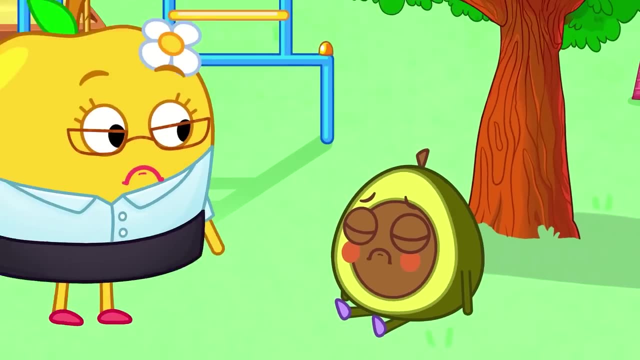 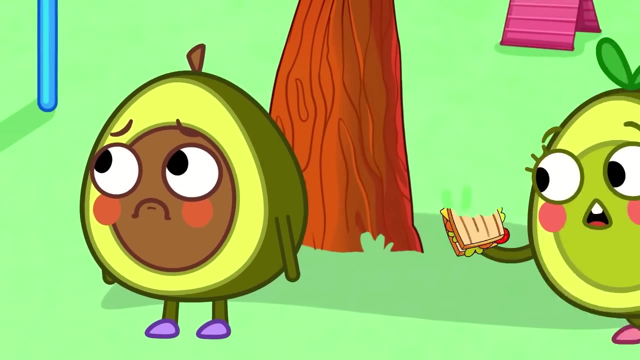 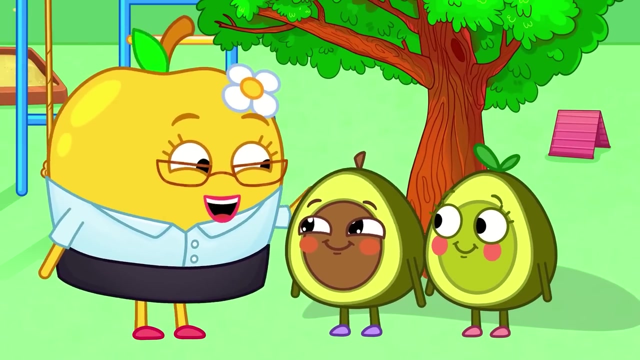 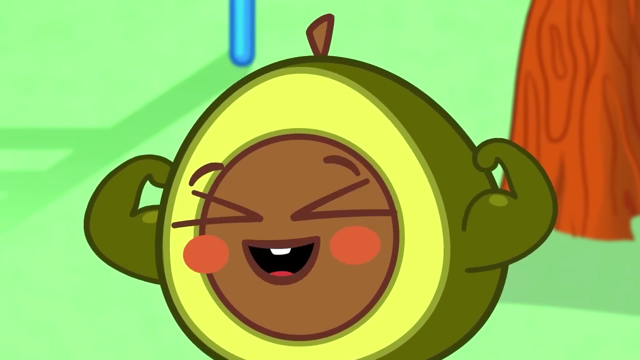 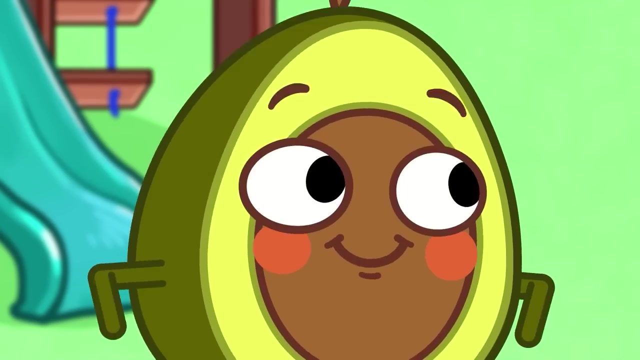 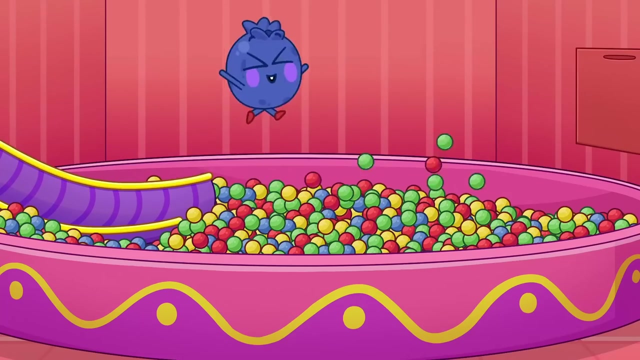 You need to eat it. You need to throw it. Pit has no energy left. Are you hungry? Penny saved some sandwich for you. It'll give you energy. Healthy food make us stronger. It's just a perfect face. every day We have a hundred new friends. And you will never bring me a neverending family. I could take it. I could take it. Suddenly, we decided to begin a family. This is what I call an environment structure is there all the time. This is what I do all the time. 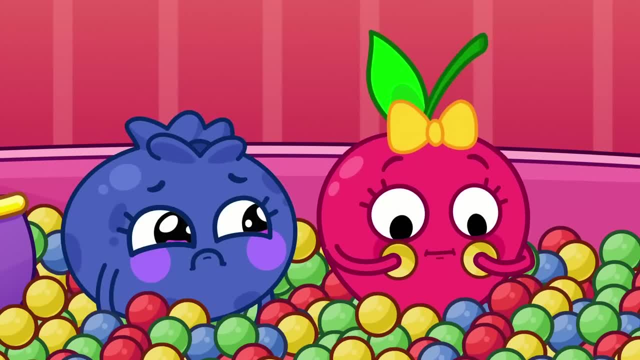 Be patient. I'm seaweed for your entire life. Get some strawberries. Whatever you get, I have dominion His days with court. Whatever you get, I get EK. Is he here for the music Or something else? Hen? why are you here all the time? 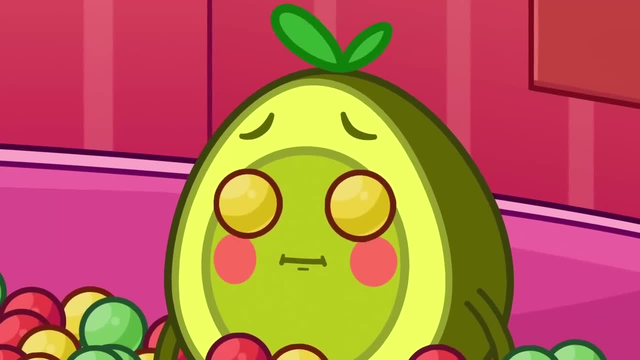 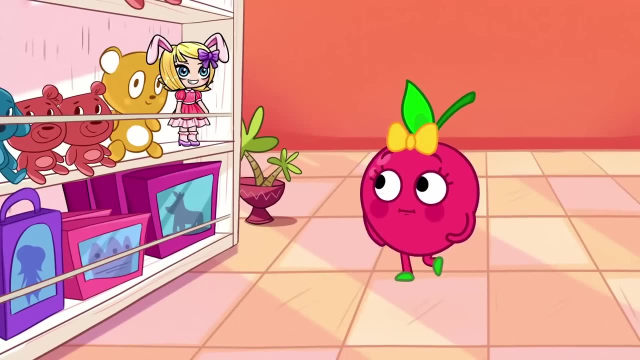 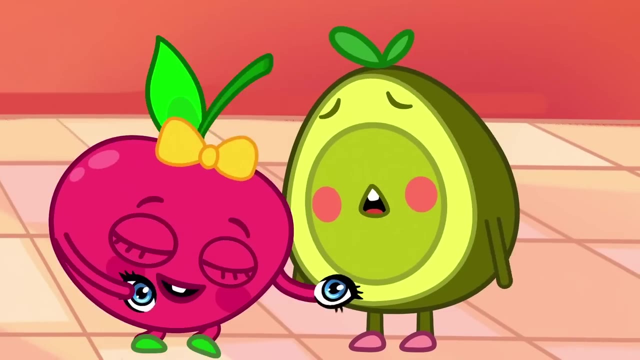 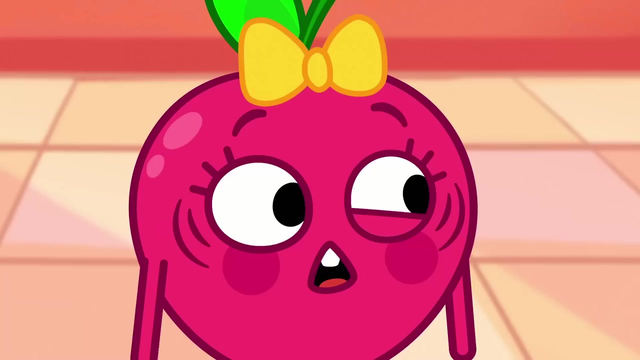 Jack's fucking balls are up on the stage. I could go play football too. No, those yellow balls aren't eyes. Are there any eyes over here? The doll's eyes might work- Now Penny can see, But they don't look like Penny's eyes. 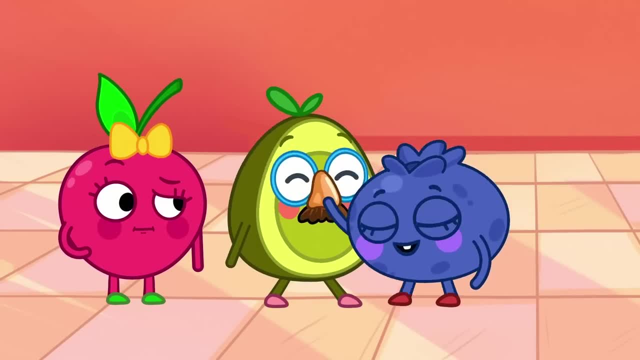 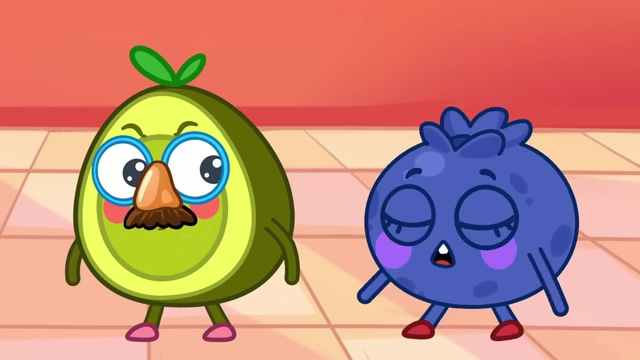 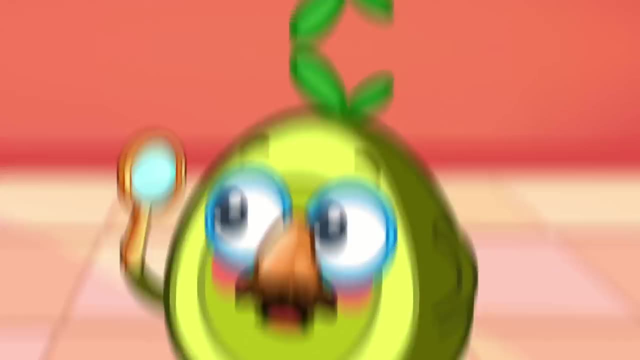 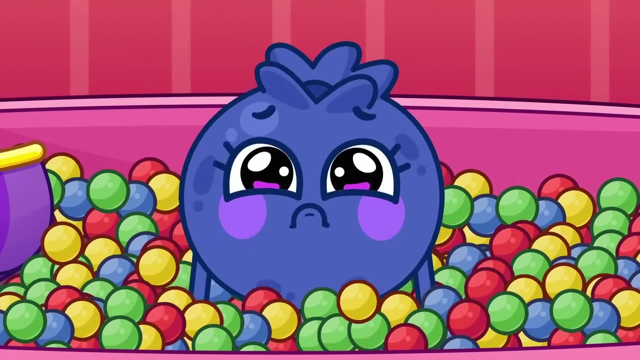 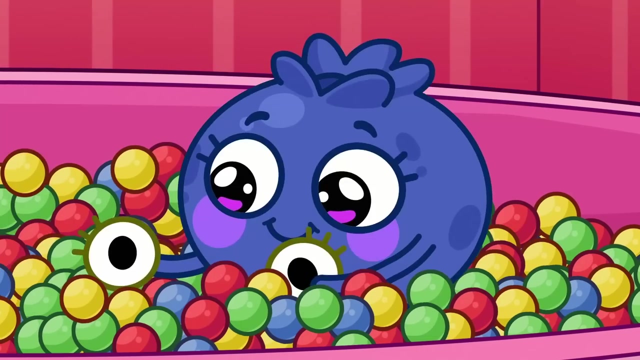 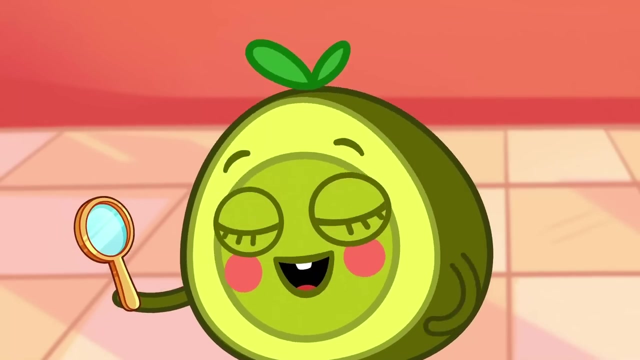 Blueberry found some eyes. Try them on Penny. Oh, those are too silly. What do you think Penny? Watch out Blueberry. Watch out Blueberry. I see Penny's eyes. Yay, Penny has her eyes back. 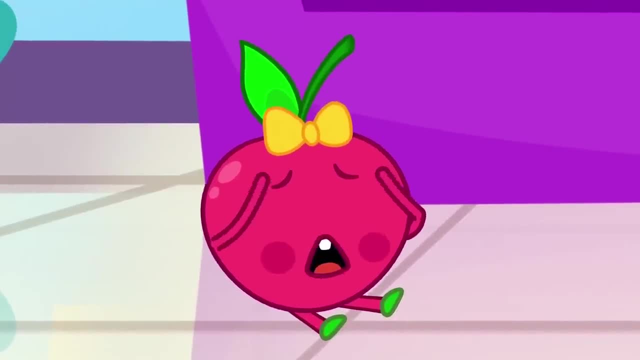 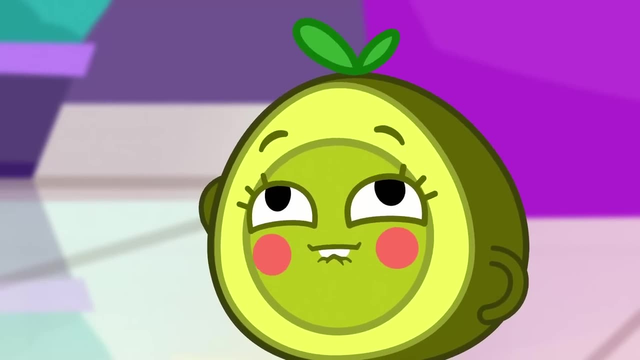 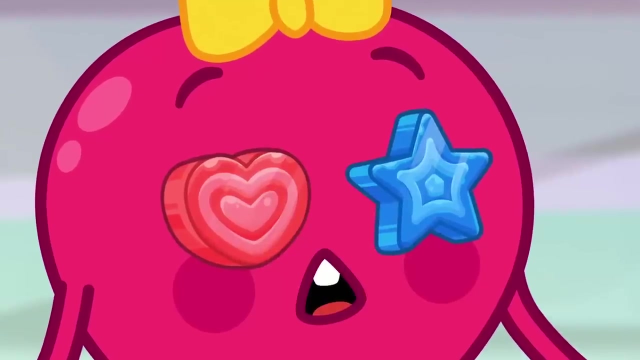 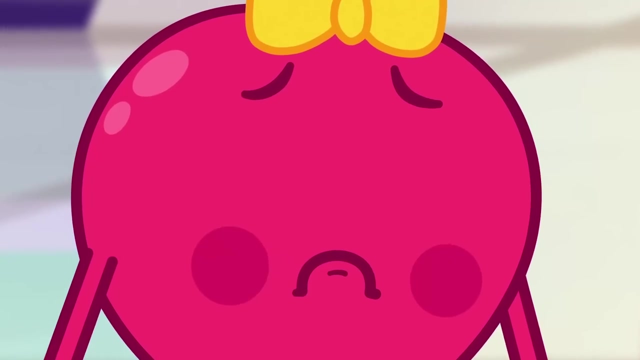 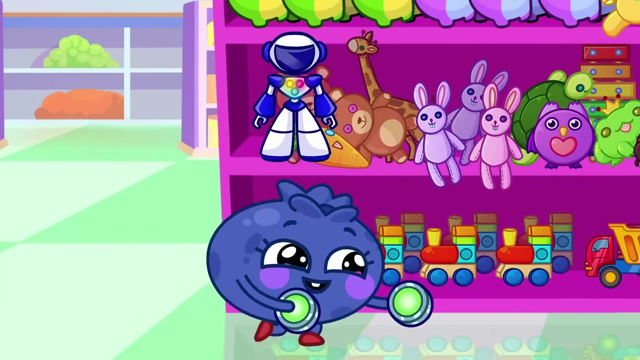 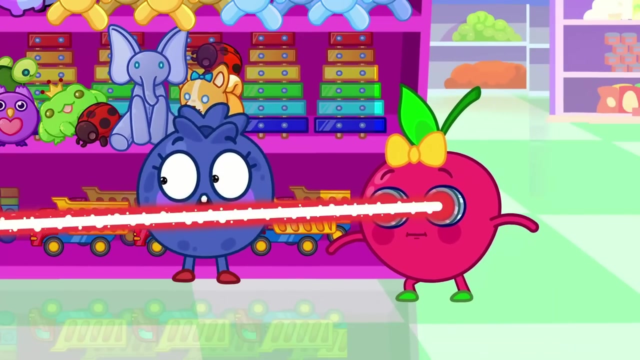 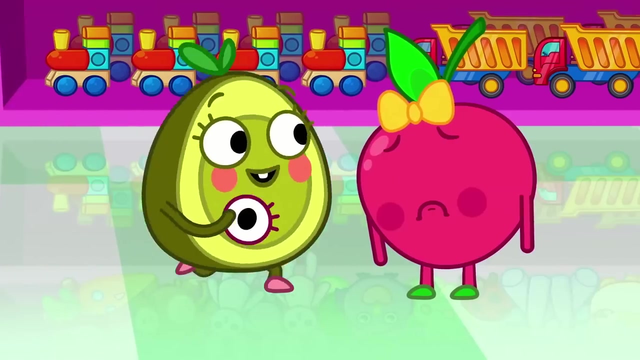 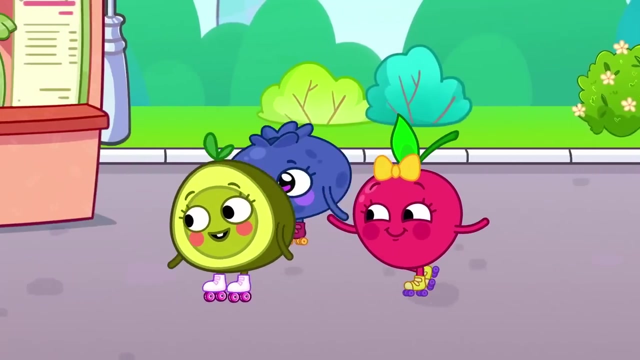 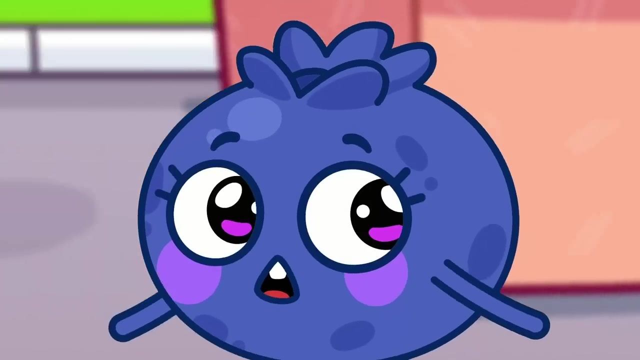 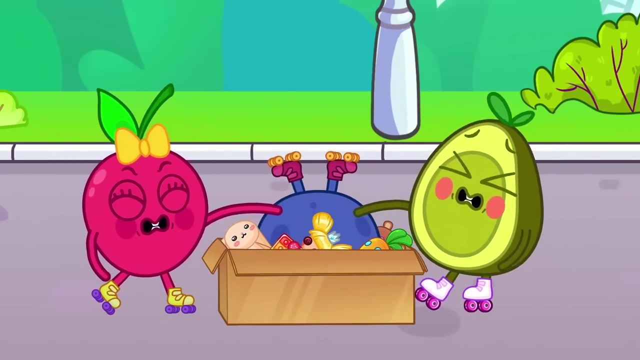 Cherry lost her eyes. Where are my eyes? Oh, Penny, those are not eyes, They're toys. Maybe robot eyes would work. They shoot laser beams. Those are Cherry's eyes. That's much better Now. Blueberry lost her eyes. 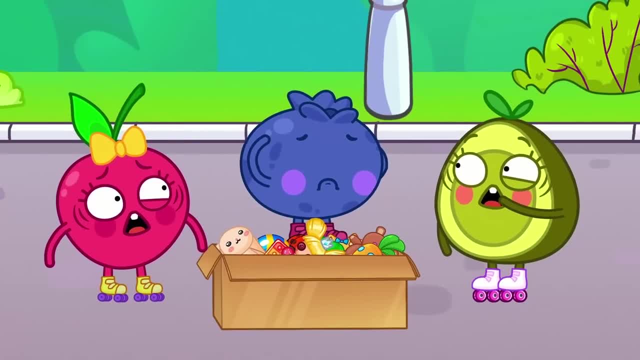 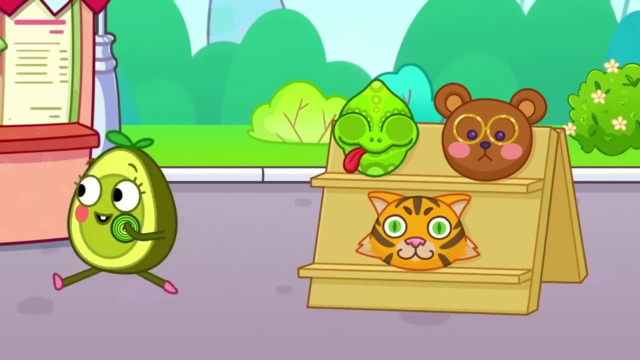 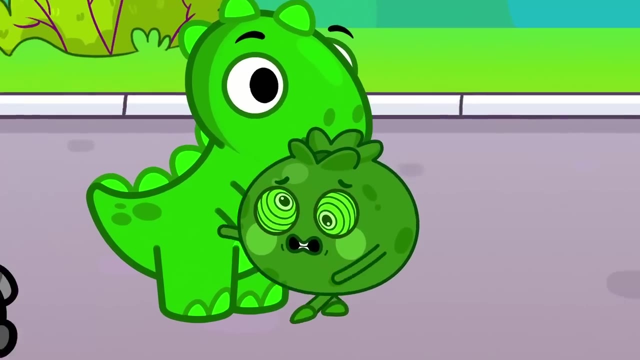 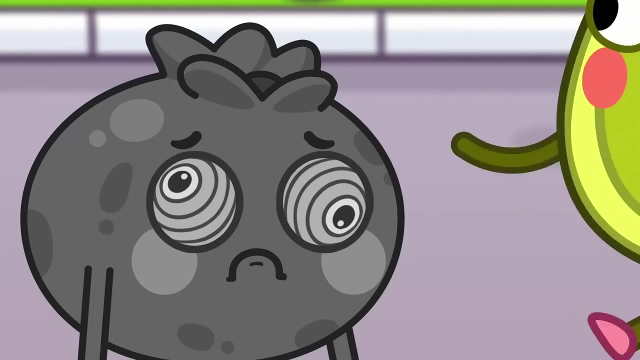 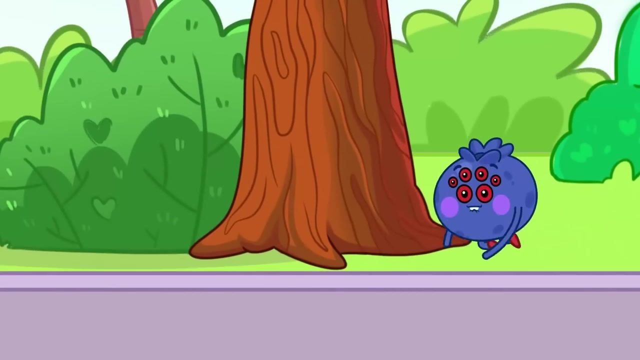 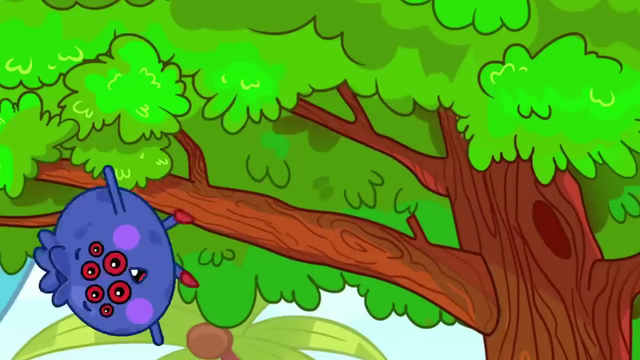 Where are my eyes? Are they? Let's try the Lizard eyes. Blueberry is now a chameleon changing colors. Will Spider-Eyes work? Now she's a spider, Oh no, Whoa, Whoa, Whoa. 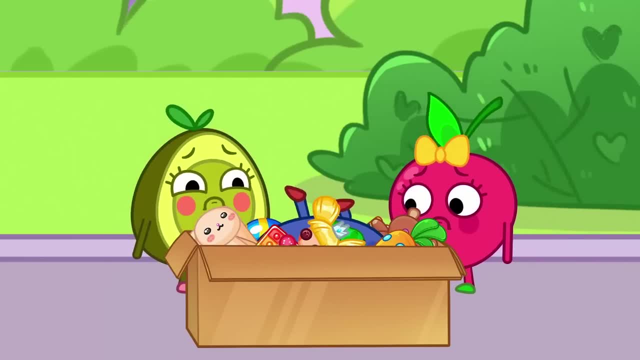 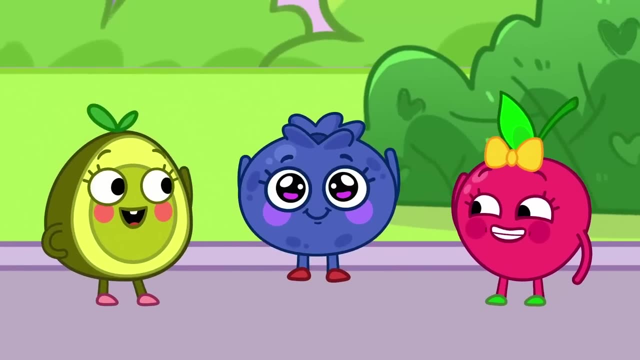 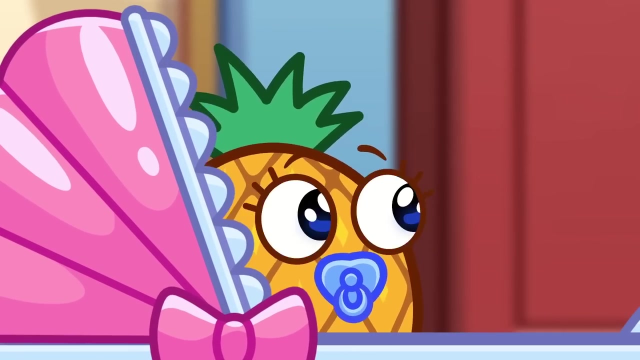 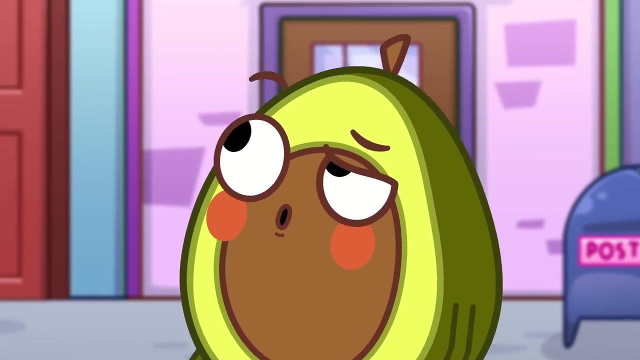 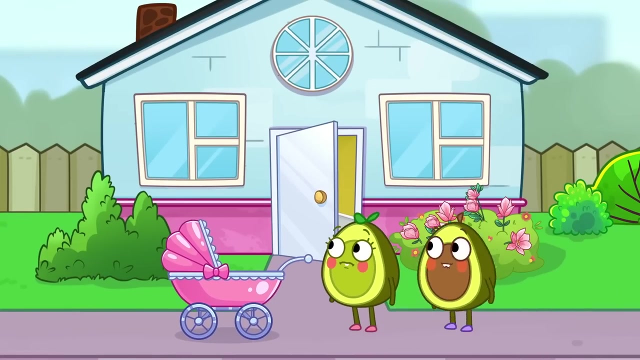 Whoa Oh, Blueberry got her eyes back There. everyone is back to normal. Pit and Penny found a baby in a stroller, Shut up on his mom. Gotta find his mom. Where should they look first? Maybe the baby's mother is here. 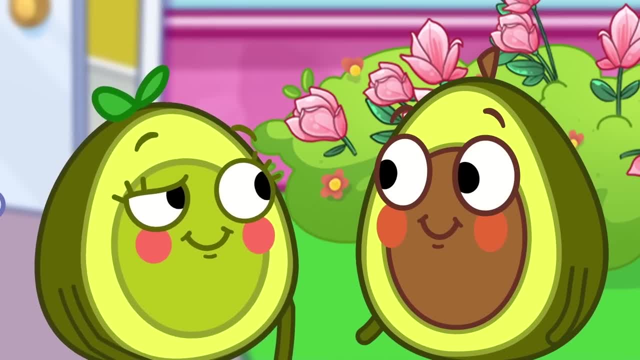 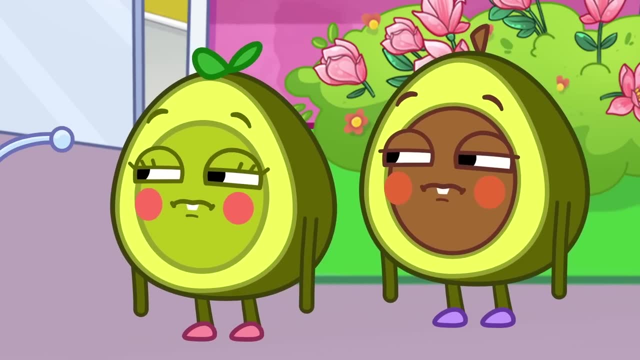 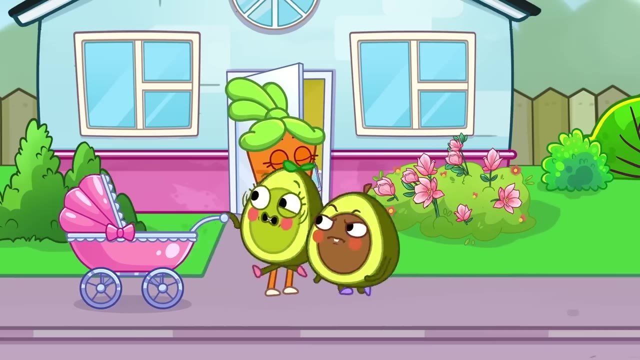 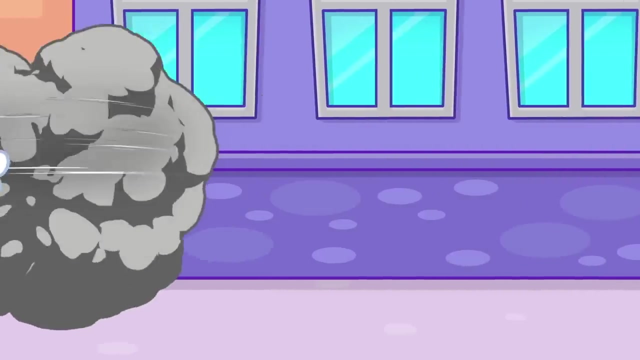 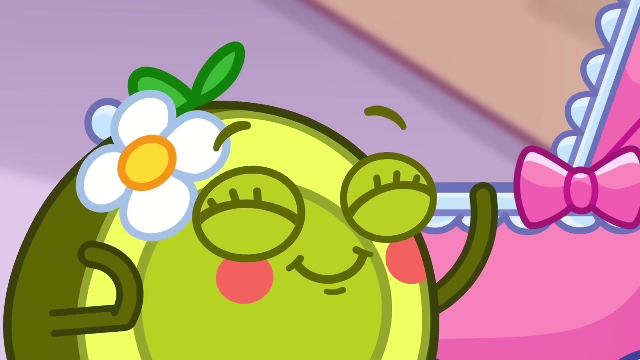 It's Carrot's baby. Is this your baby? You'll have to keep looking. The police will help us, But Pit and Penny don't want help. Someone stole Miss Apple's flower. Oops, it was Penny, It's mine. 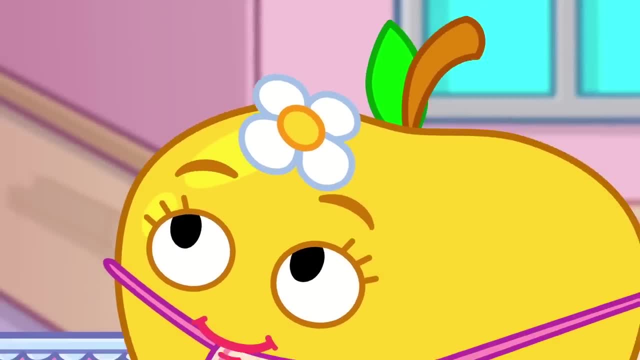 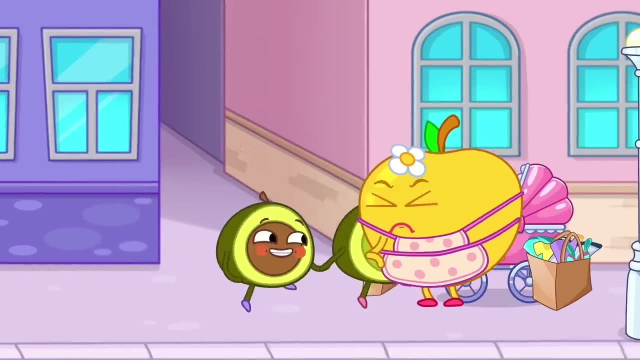 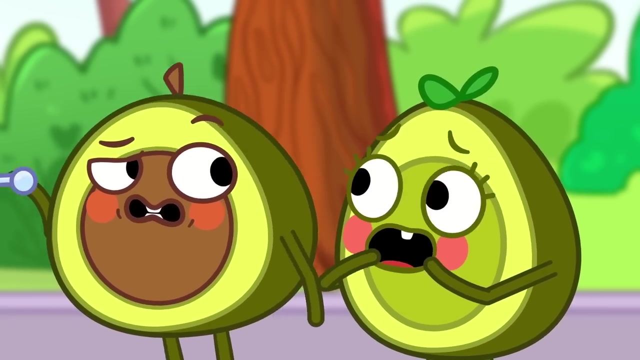 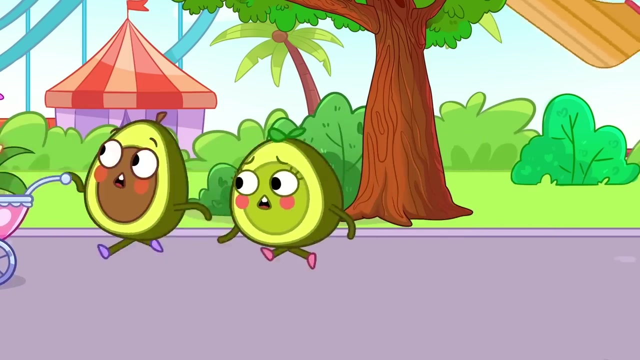 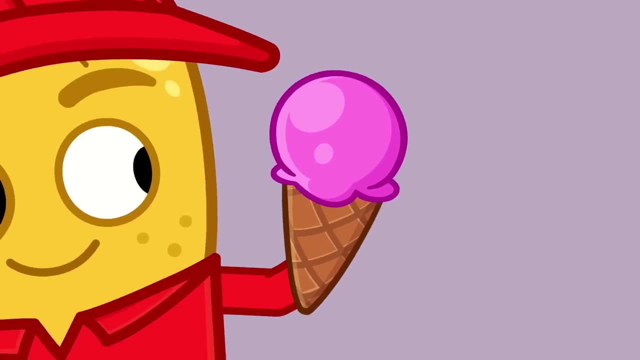 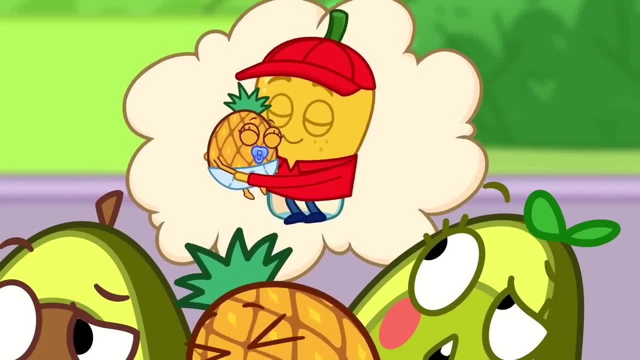 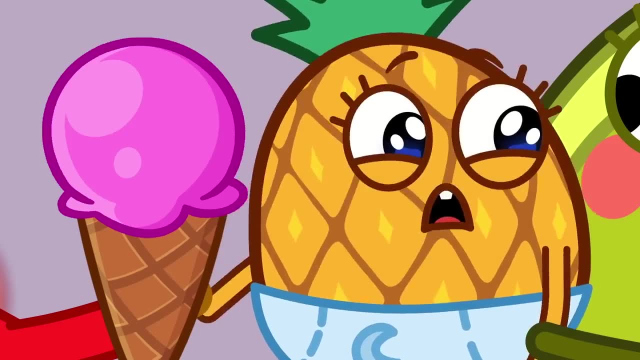 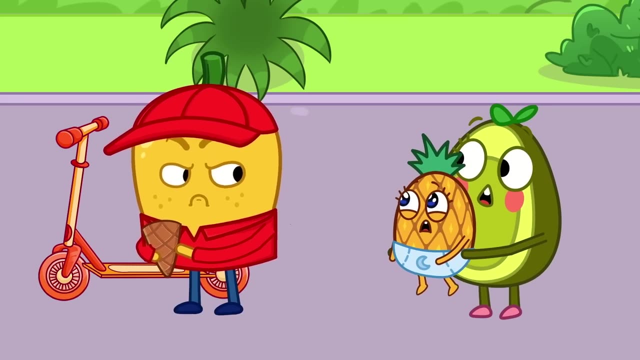 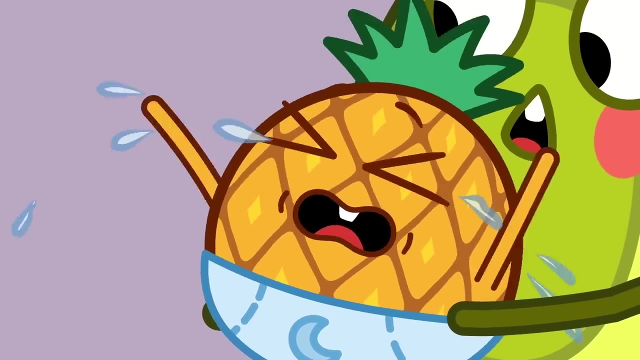 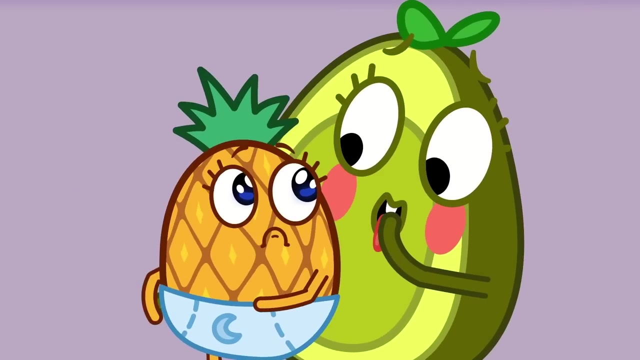 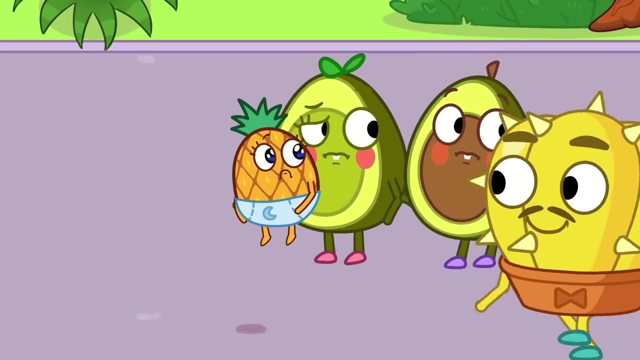 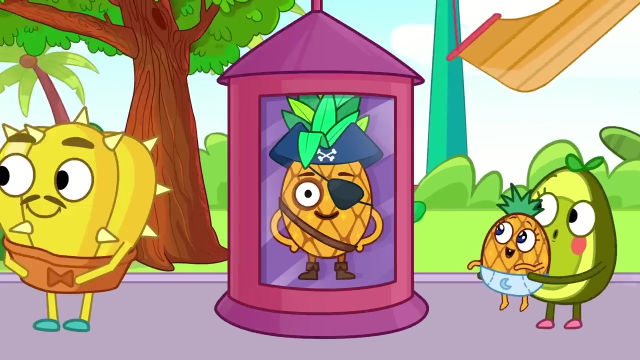 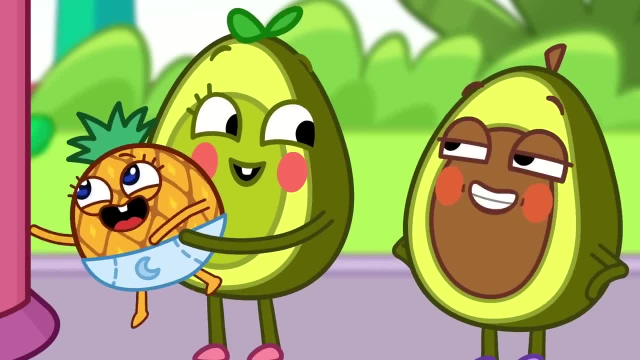 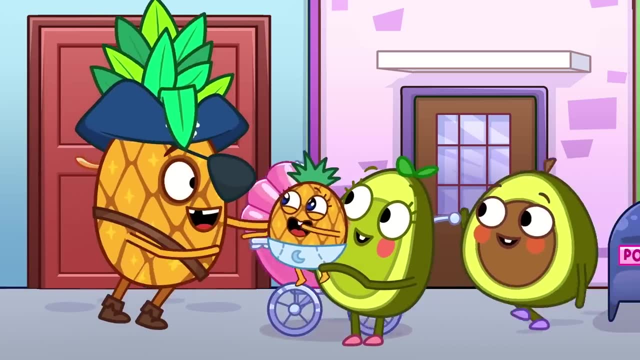 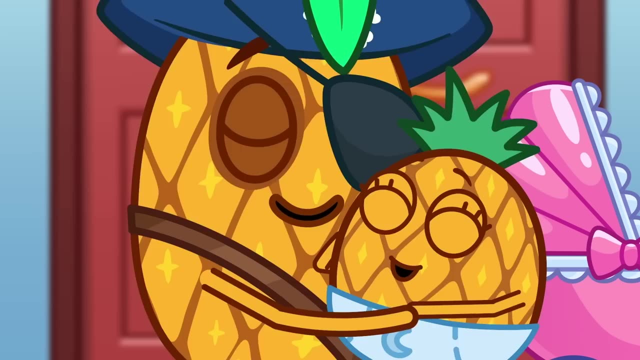 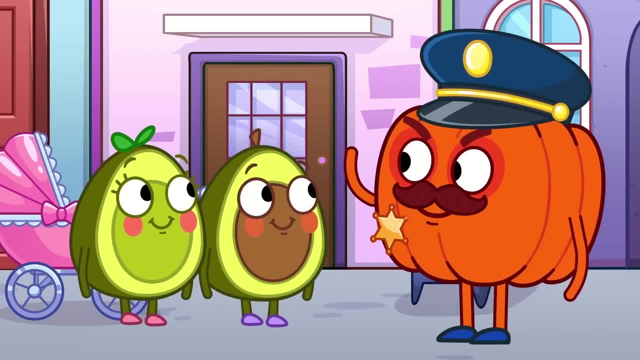 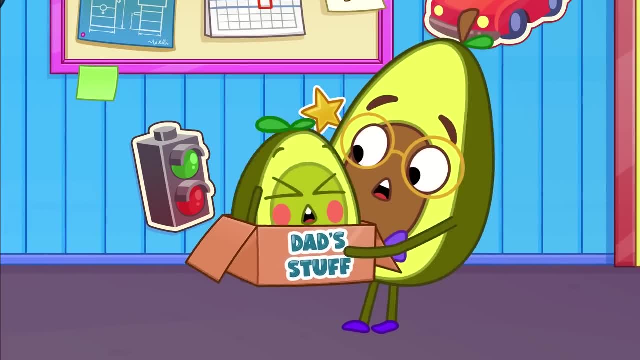 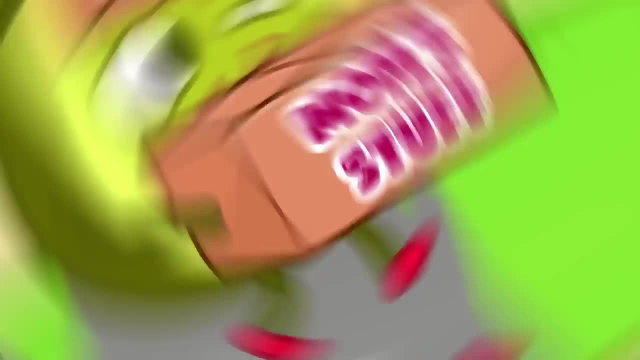 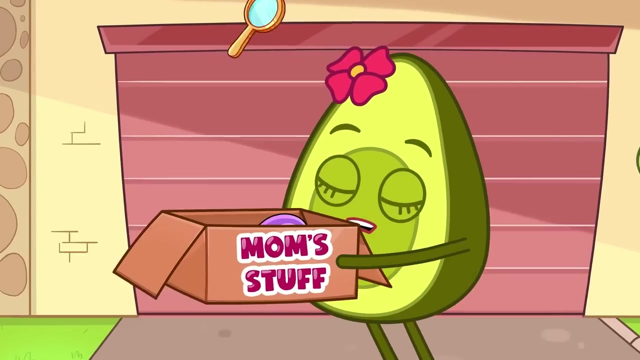 If you find lost children, please call the police. They promised Daddy's busy cleaning the garage. Patty isn't there. Aha, I found you, Patty. Mommy is also busy cleaning Kids. you have things to do too. 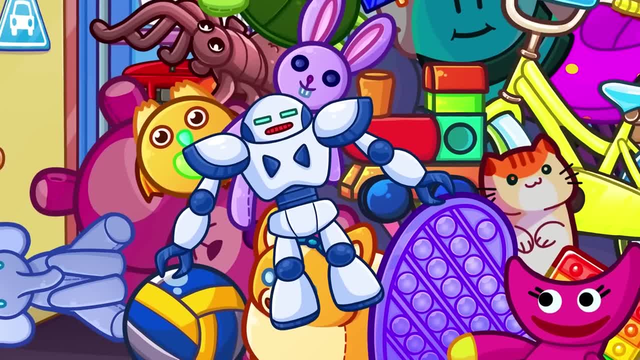 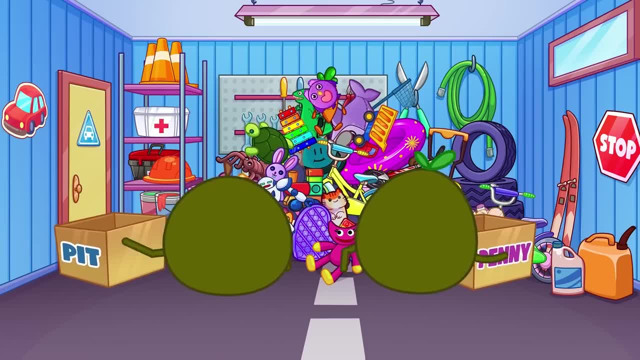 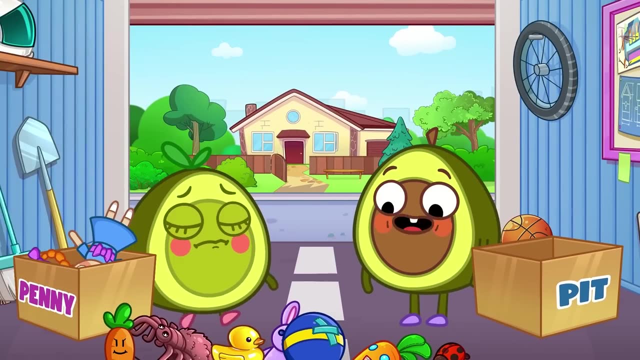 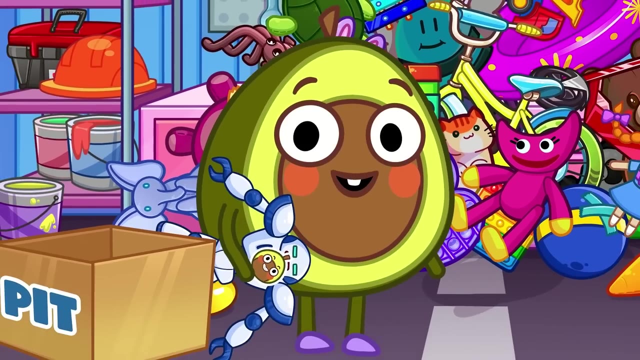 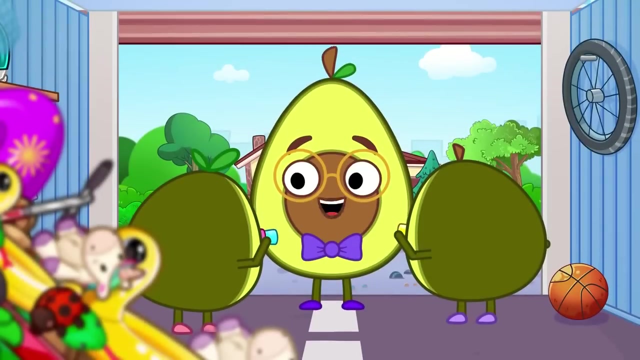 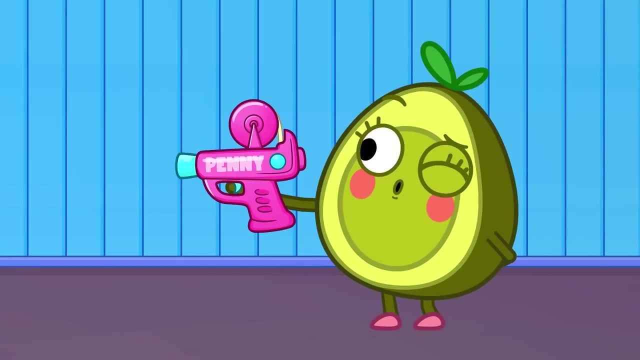 You have to clean up all your toys. Why is this so boring? Look, Daddy has sticker guns: One for Penny, one for Pit Mark- the items that belong to you. This will be much more fun. Ha Ha Ha. 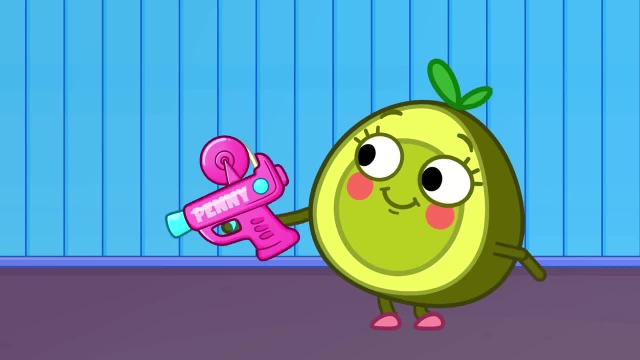 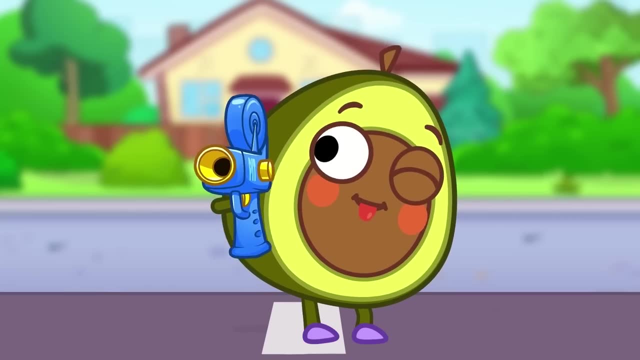 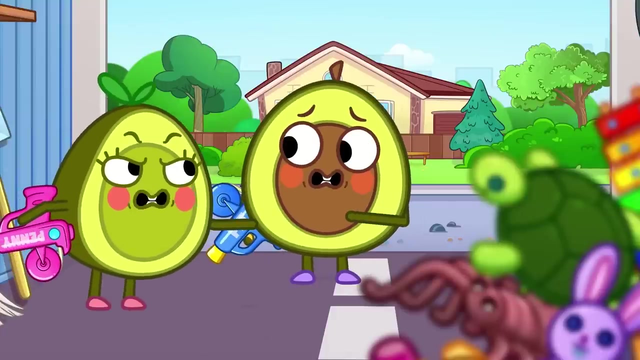 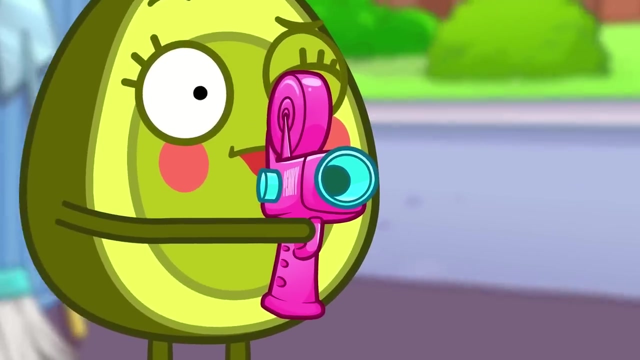 Ha Ha Ha. Good shot, Penny, You try Pit, Can he hit the bike He missed? Hey, That's mine, My sticker. Now it's mine, Penny, that's Pit's bike, What, Okay? 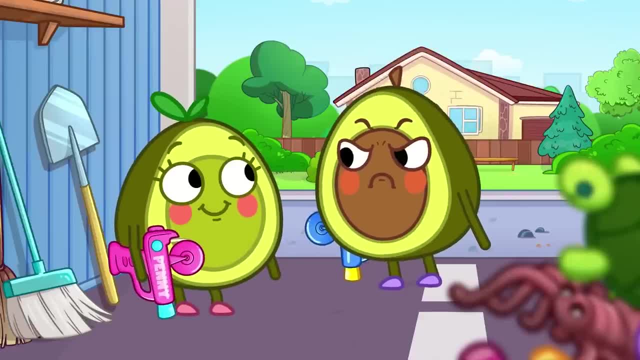 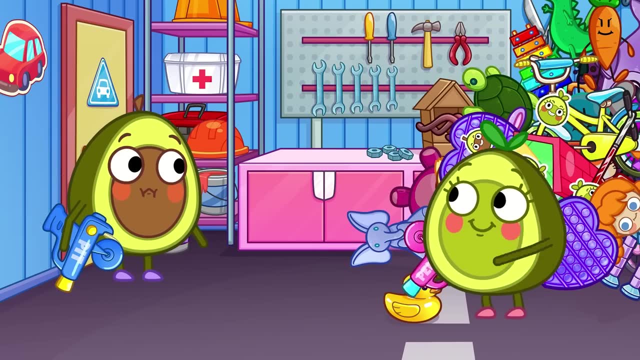 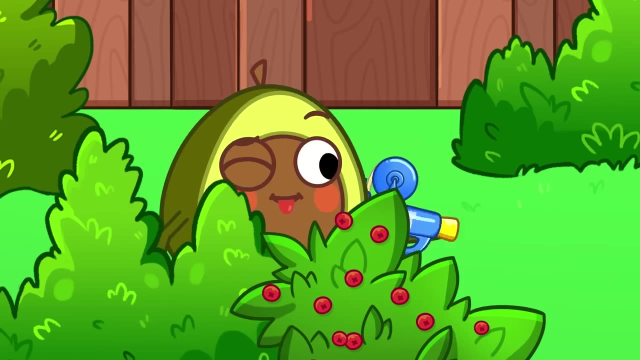 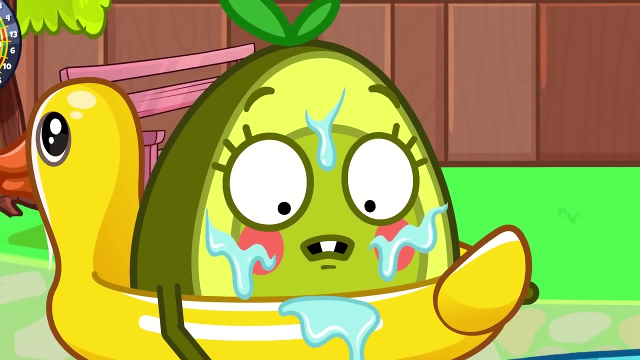 My sticker. Then this is mine, The door is mine. Patty wants to play in the pool? Yay, Yay, The pool is mine, Yay, Oh, yeah, Ah, Ah, Ah, Ah, Ah Hmm. 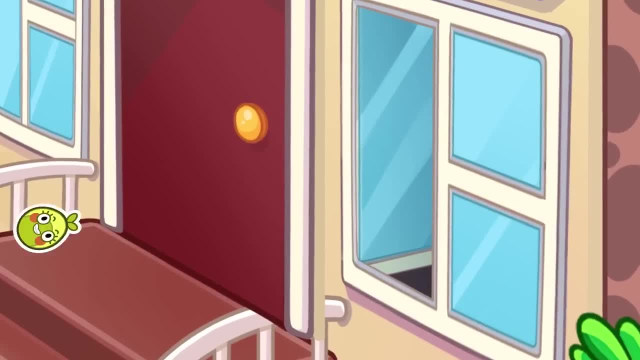 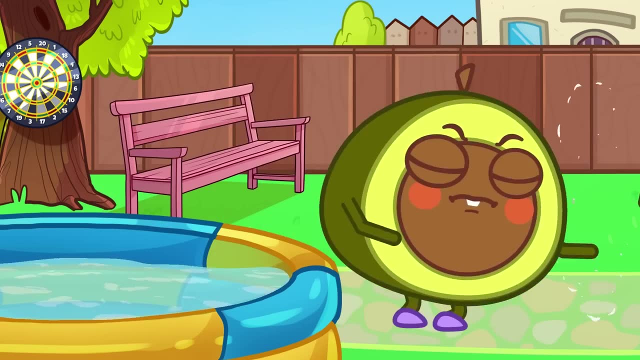 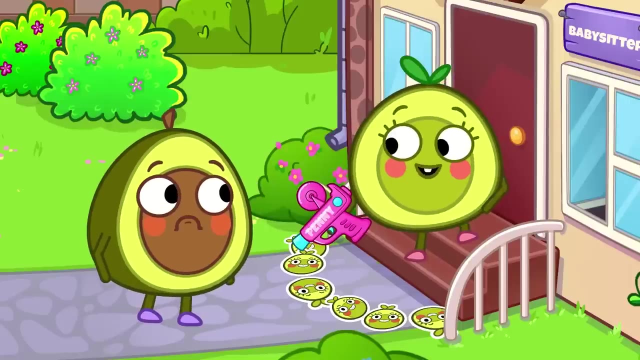 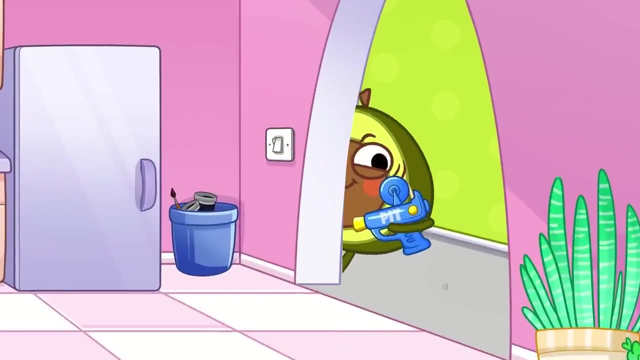 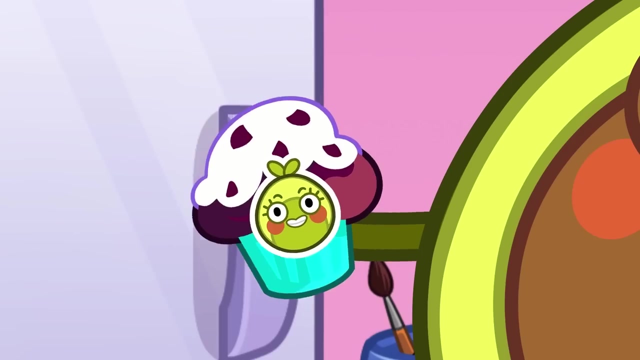 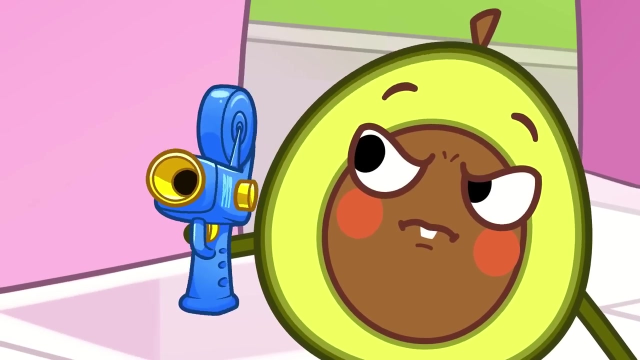 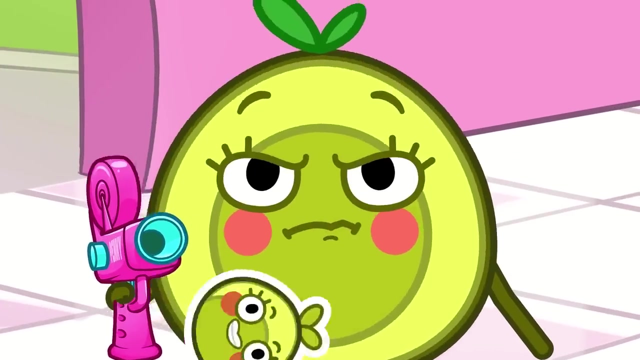 Hey, Huh, Hmm, Hmm, Hmm. That's the bedroom door. Now our room is mine. This part of the backyard is mine. Pete is very angry, But he has a plan: A banner sticker. The cake is mine, Now it's mine. 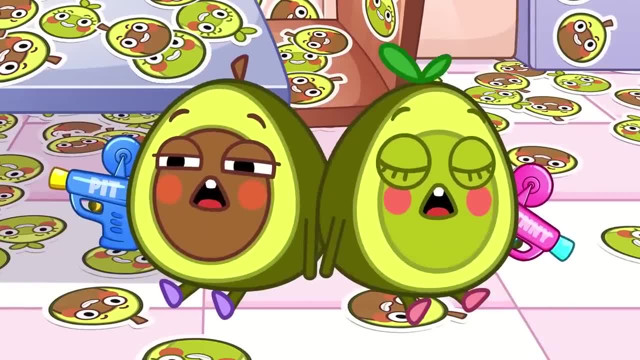 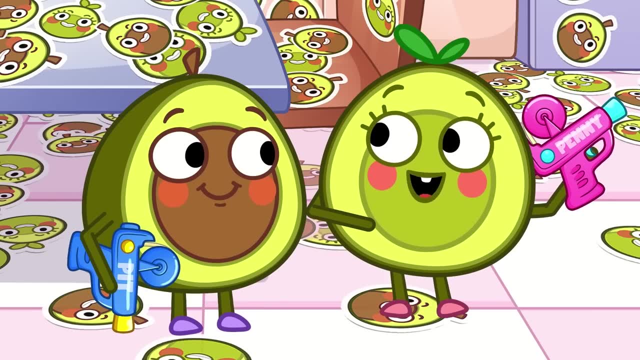 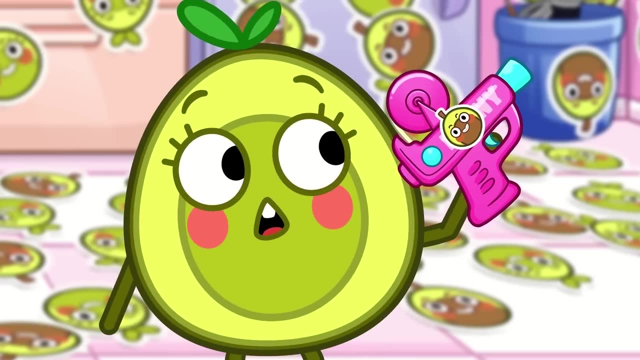 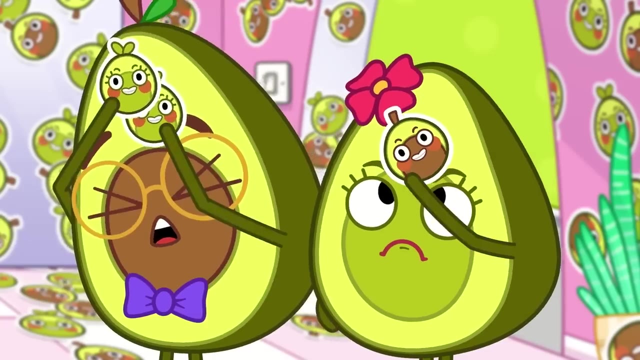 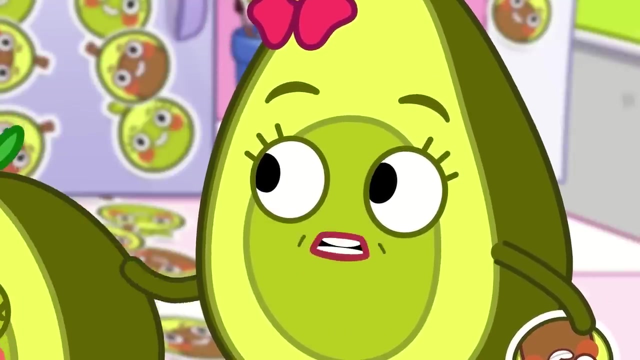 Everything is covered in stickers. Kings, what happened? Huh, Oh, Aha, Daddy is mine And mommy is mine. Pani, that's now bed sticker gone. Oh, Oh Awww. Kids, there are things that cannot be divided.